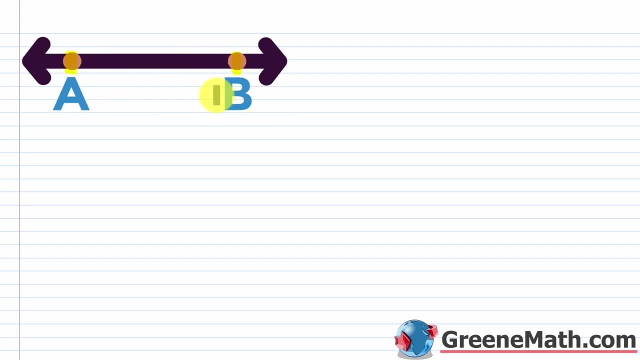 you'll see that you have a point A and also a point B, So those two distinct points can be used to determine a line. So you see, we've drawn a line through them. We can also use those letters, the A and the B, to name the line if we want. So we can call this line. 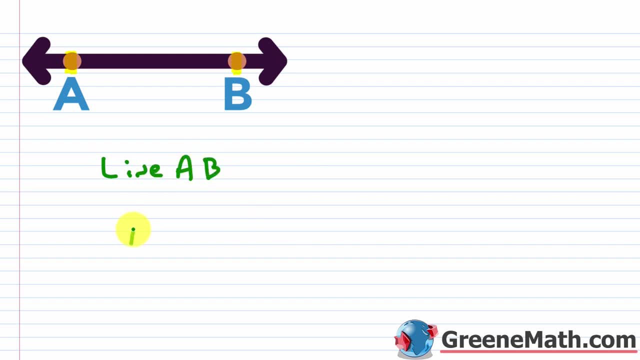 AB like this, or we can also put the AB and we can put a line on top, like this. Now I want you to notice that you have arrows at each end and that tells you that the line continues indefinitely in each direction. 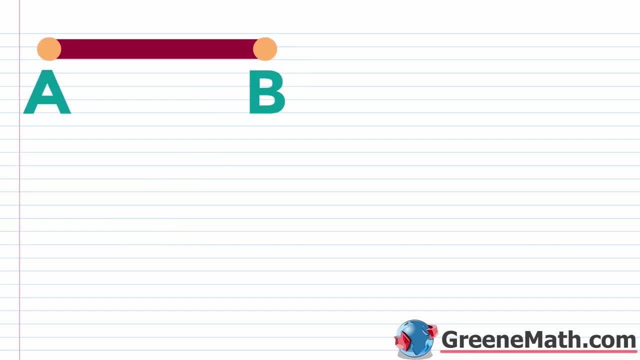 Now, similarly, you have something known as a line segment. With a line segment, it's just a piece of a line or a part of a line. So notice how you have an end point here with A and an end point here with B, So here it doesn't continue indefinitely. 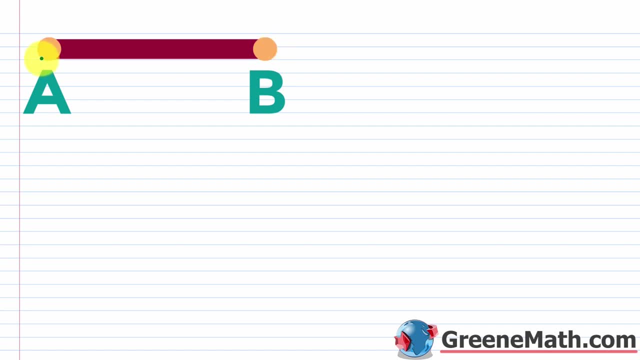 in each direction. It's a finite or countable length from the point A to the point B. So this is your line segment. your line segment AB. Okay, And you can also write it like this: You can put AB with a little line on top and you're not going to have arrows there, It's another line. 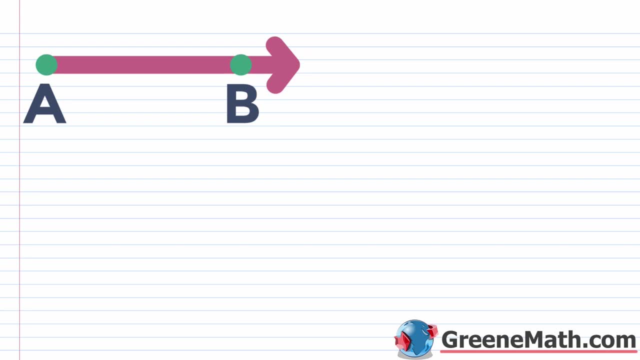 segment that's put on top of AB. Okay, Lastly, we're going to talk about the concept of a ray. So here you have one end point. Okay, In this case it's going to be A and it's going to extend through this point B indefinitely. Okay, 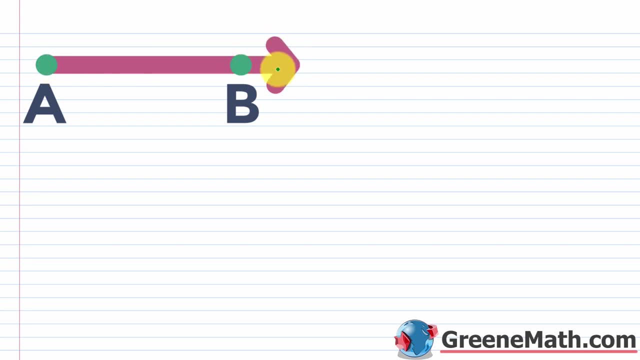 So we see this arrow here. It tells us that it starts at A and continues through B indefinitely. So this is going to be the ray, the ray AB, or you could write AB and you can do this Alright. so now I want to talk about an angle and 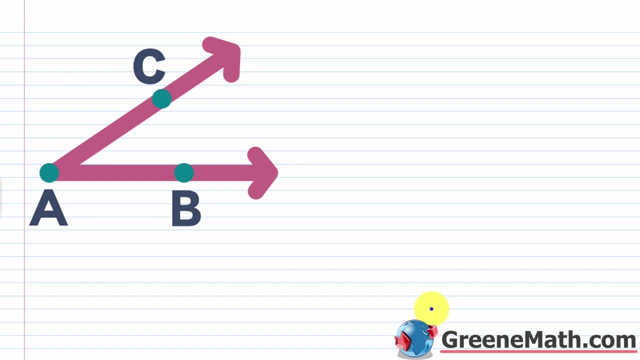 basically, an angle consists of two different rays with the same end point. So when we talk about the two rays, these are the sides of the angle and the common end point is the vertex of the angle. So if we look at our example here, we have a ray. 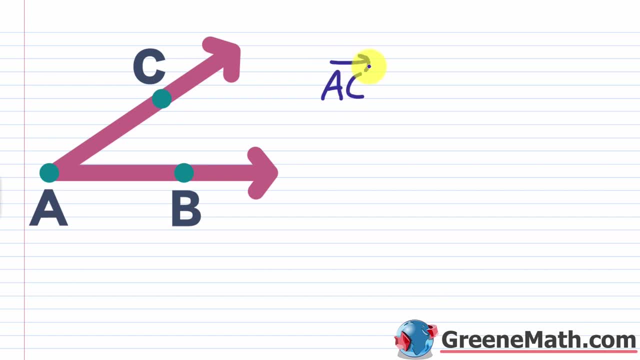 AC. So we have a ray AC and then we have another ray which is AB, So another ray which is AB. So these are going to be the sides for my angle. Okay, Additionally, A is the common end point, so that's my vertex. Now, if I'm naming the, 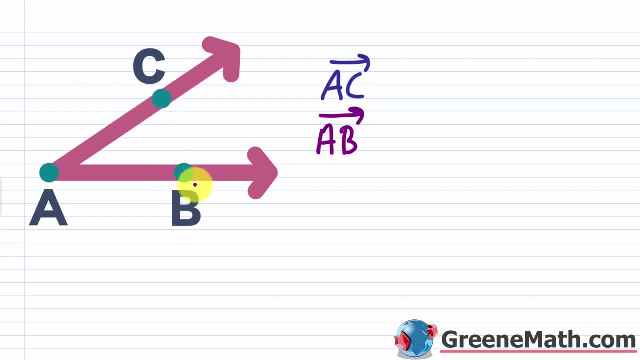 angle, then I can call it angle CAB. You can go in order like that, or you could go the other way. You could say angle BAC, okay, Or you could just use the letter of the vertex. Now we can write out angle each time, or you can use: 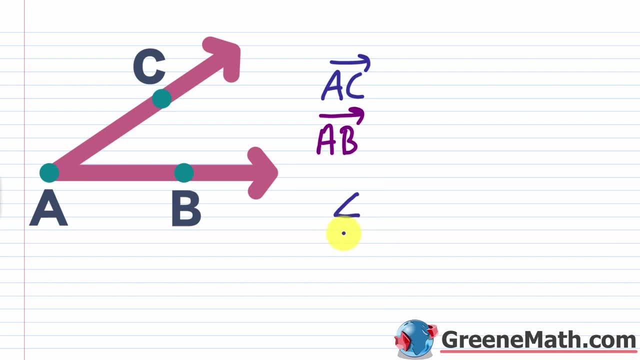 this special symbol, So you can use this symbol here and I could say: okay, this is angle CAB or it's angle BAC. Okay, notice how A the vertex is in the middle each time. And then also I could 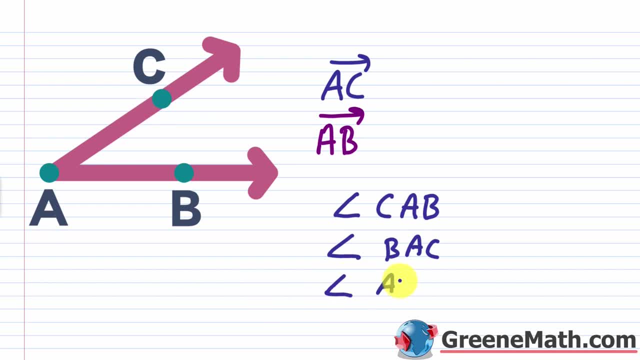 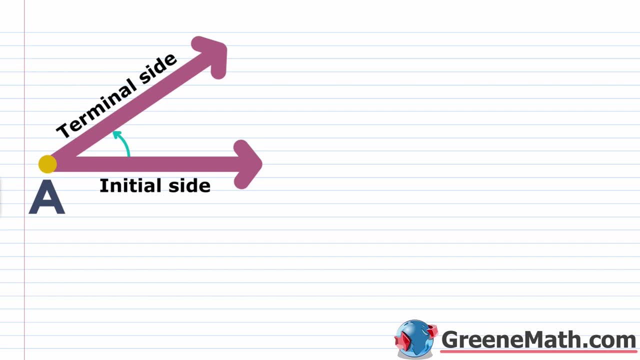 just use the letter of the vertex, So I can say this is angle A. Alright, now associated with every angle is going to be its measure, which is generated by a rotation about the vertex. So the measure will be determined by rotating a ray starting. 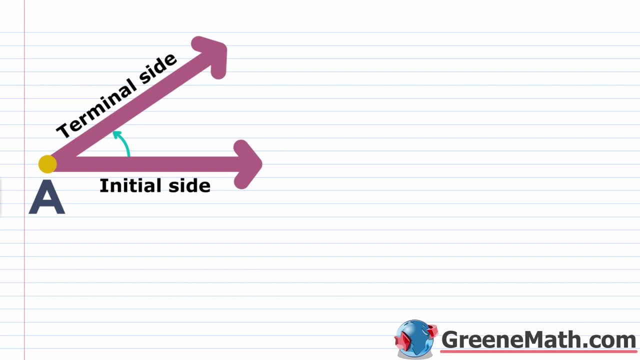 at one side of the angle, which is called the initial side. So let me just highlight that, For in this case, the initial side is here. We'll talk more about the standard position later on in the course. For right now, our initial. 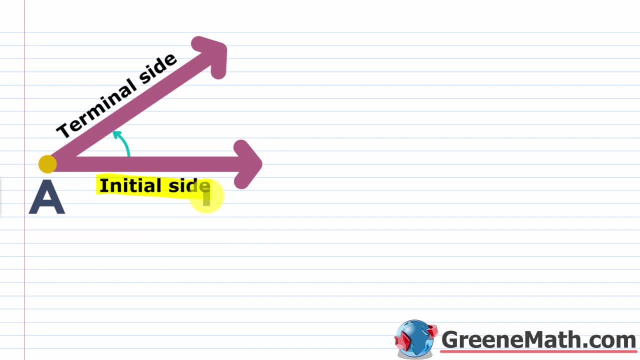 side is going to be right there. Okay, So that's the starting position, and then we rotate to the other position on the other side, which is known as the terminal side, which, in this case, is right here. So you can imagine that you started with two rays that are on top of 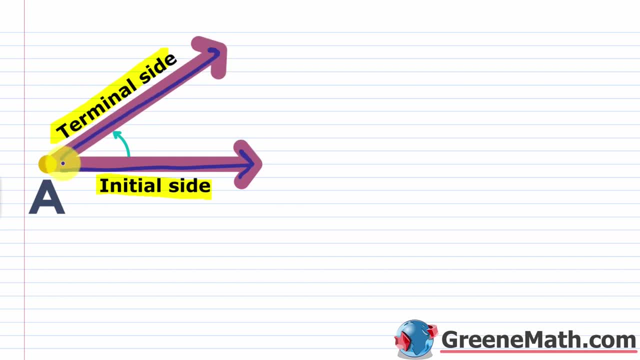 each other. So this guy represents this guy in the end, and I know I'm not drawing that perfectly well, but basically you can think about starting here and then just rotating about the vertex to get here. So this is your initial side, where the two are on top of each other, and then it rotates. 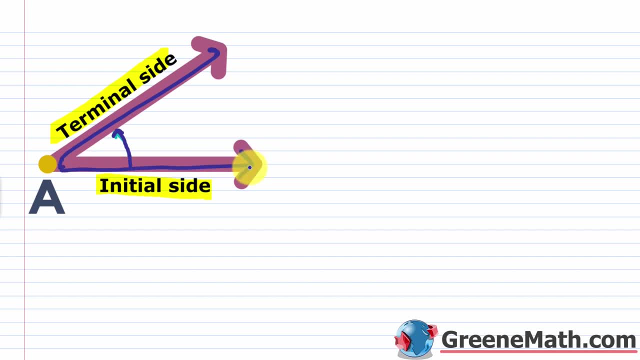 to the terminal side, where you still have one ray here or one side and then another ray up here. Now, when we rotate in a counterclockwise direction- so meaning I start here and I rotate this way- okay, that's how I'm measuring- well, what happens is I generate a positive. 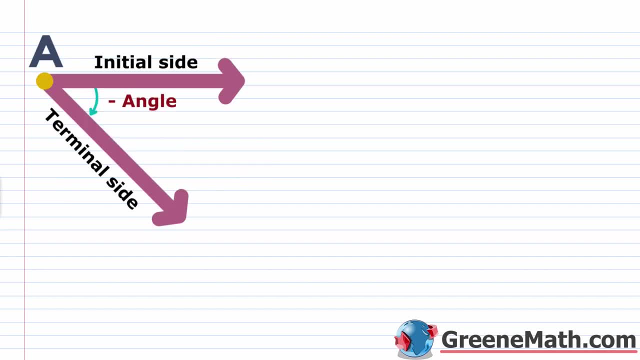 angle. Okay, Now if I go the other way, if I go clockwise, I'm going to generate a negative angle. We'll talk more about this as we progress through the course. but basically, if I started this way and I went that, 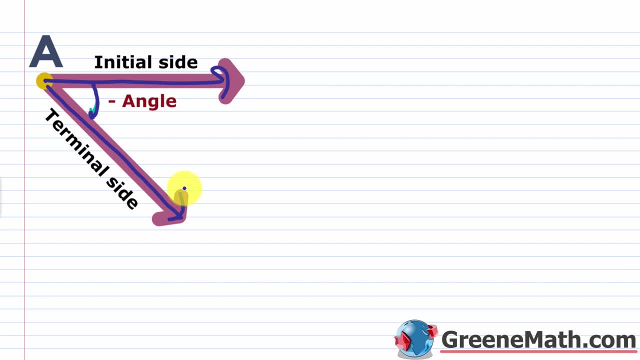 way. okay, now I'm generating a negative angle. Now you can imagine if I started here and I went this way around to generate the same terminal side. okay, well, now I would have a positive angle because I'm going counterclockwise. 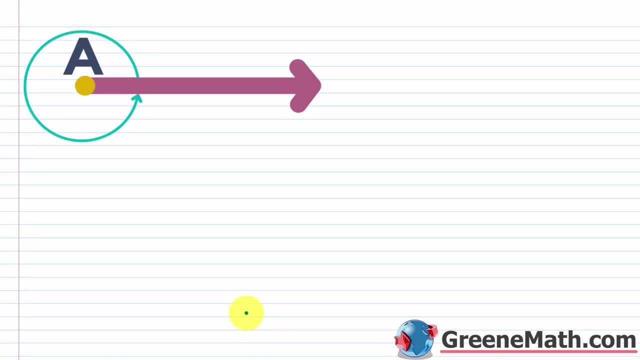 for the rotation. Okay, so we'll talk more about this as we progress. Alright, so when working with angles, we're often going to measure our angle using the degree. Okay, so this is a unit of measure for us. We'll also see radians here shortly, but for now, when we work with the degree, 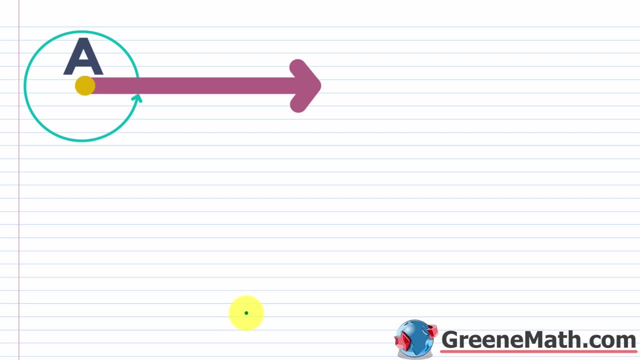 we assign 360 degrees to one complete rotation of a ray. So in other words, what we're saying here is that the terminal side of the angle will correspond exactly to the initial side when it makes this complete rotation. So you can see this image that we have here. 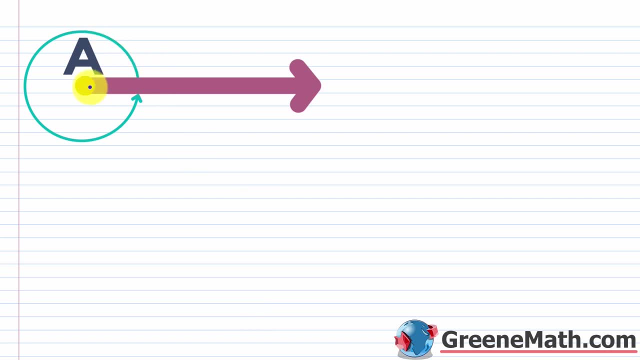 and you can imagine that we started out with two rays that were on top of each other, okay, and then we rotated it completely around, So it's one complete rotation here, and we assign the value to that angle: 360 degrees. Okay, so that's. 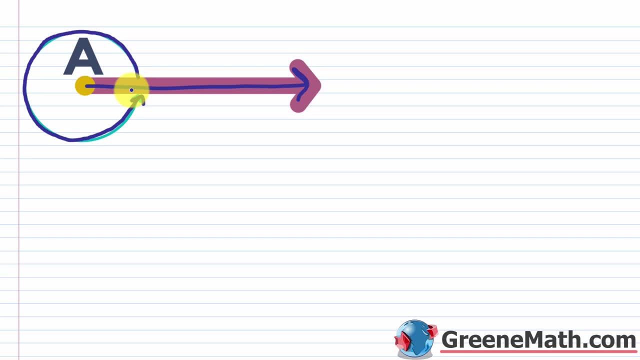 one complete rotation. Now, of course, you're going to have a lot of scenarios where you make more than one complete rotation or less than one complete rotation. So if, for example, you made 1 over 360, that amount of a. 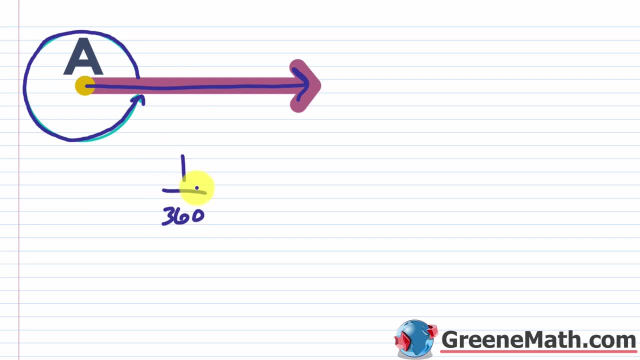 complete rotation. well, we would just take this number in the numerator here, which is 1, and we would say that we have one degree in this case. okay, We can also write this using our degree symbol, so we can say: it's one degree, like that, If you had, for example, 5 over 360,, okay, that. 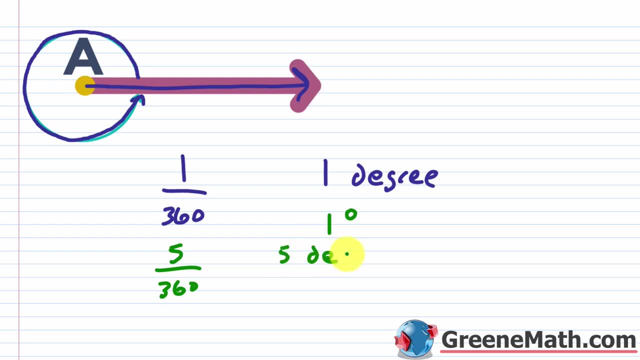 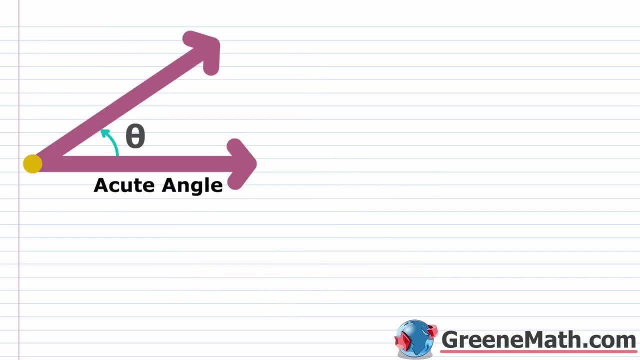 amount of a complete rotation. this would be now 5 degrees. okay, That would be the measure of that angle, and you can, of course, still write it like this: 5 degrees. Now, when we work with angles, we're going to have some terminology that we have to get used to. So the first guy we want to talk, 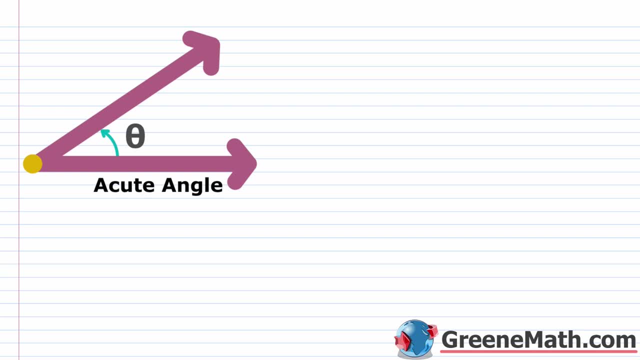 about is an acute angle. okay, So this is where the measure of the angle is greater than 0 degrees, but less than 90 degrees. So you see, you have this Greek letter here, theta, and in trigonometry we often use these Greek letters to represent an unknown angle. 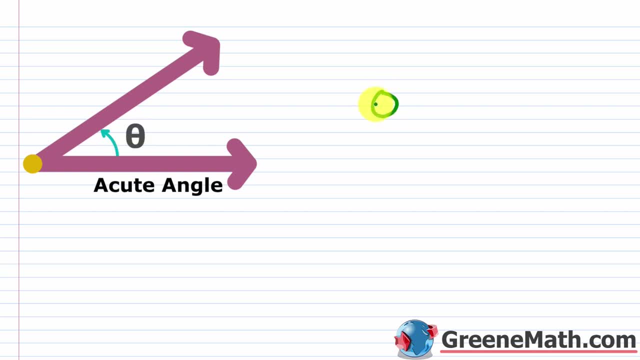 So here this is just some unknown angle. Again, theta: here we'll say that theta is greater than 0 degrees but less than 90 degrees. So this is an acute angle. Now we've all seen right angles in our algebra course, especially when you're talking about the Pythagorean formula, but a 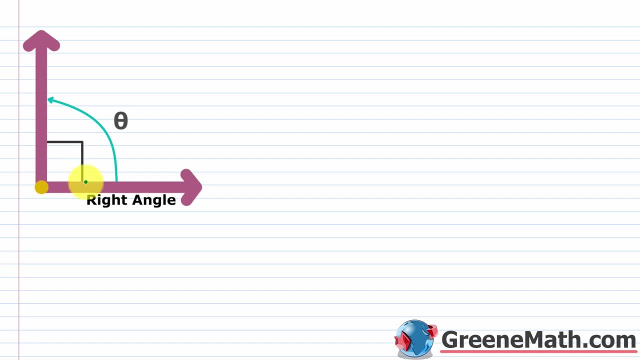 right angle. in case you don't know, you're going to denote this with this special symbol here. okay, And this is where your angle is exactly 90 degrees. okay, So theta here we can say is exactly 90 degrees. So next we want to talk about something known. 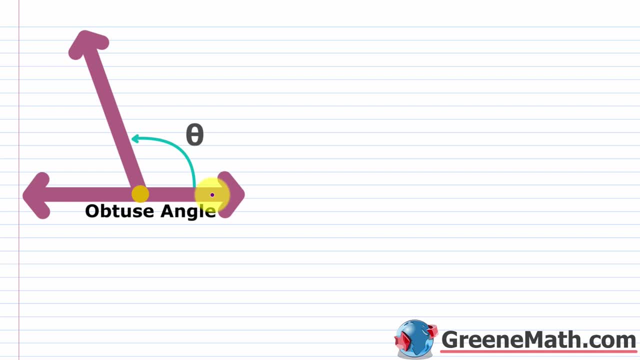 as an obtuse angle. So this is an angle that is greater than 90 degrees, but less than 180 degrees. So here we can say that theta is greater than 90 degrees, okay. the right angle, but strictly less than 180 degrees- which we'll find out in a minute- is a straight angle. So for the 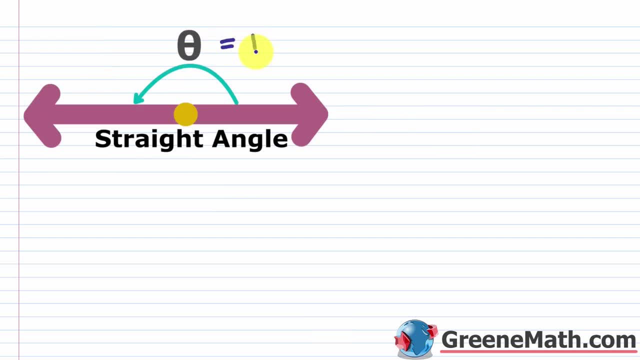 straight angle. what we're going to have is theta is going to be 180 degrees And basically what you have here. you can imagine you start out with again two rays on top of each other. you make half of a complete rotation, okay. So this guy ends up right here, okay, And you end up with what? 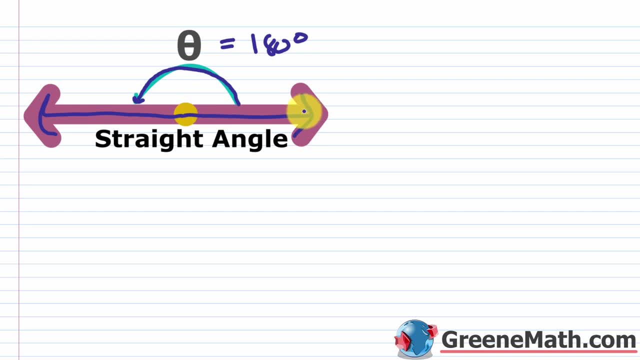 looks like a straight line, right, But basically you started with two rays on top of each other, you made half of a complete rotation and now the two rays are facing away from each other. okay, And in terms of the complete rotation, we know the degree measure is 360 degrees. 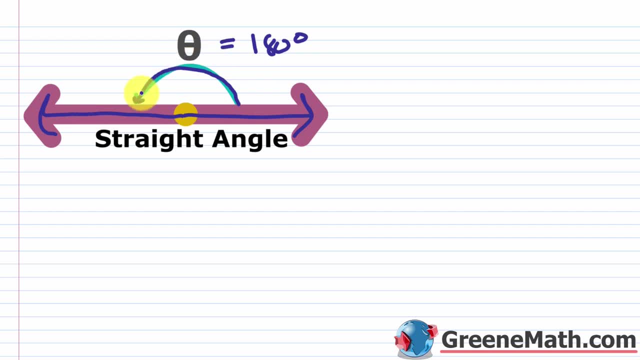 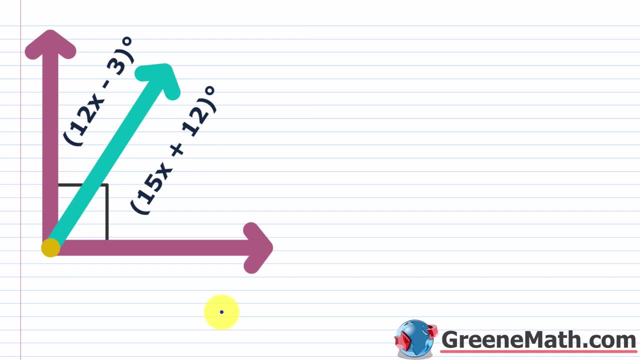 This is half of a complete rotation. So half of 360 is 180.. So that's why theta here is 180 degrees for your straight angle. All right, so let's wrap up the lesson. Let's talk about complementary and supplementary angles. So we'll start with complementary angles. 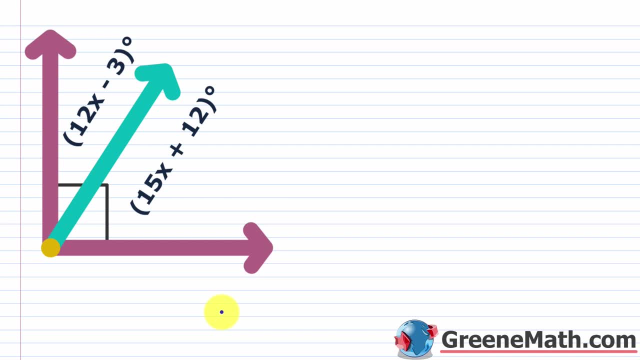 And basically, when the sum of the measures of two positive angles is 90 degrees, the angles are known as complementary angles. So here's a typical example. You can see that the bigger angle here, if I started from here and I rotated here, this is a 90 degree angle. Again, this is given to us. 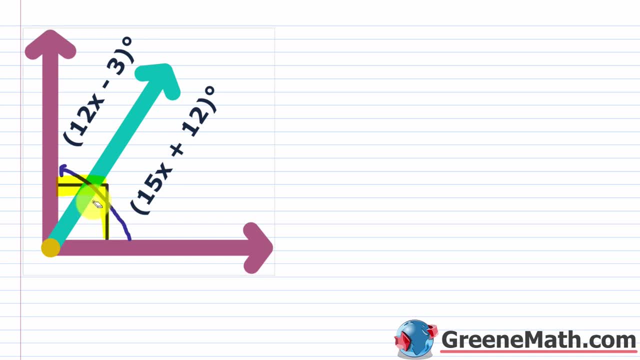 by this symbol right here. okay, But we have these two smaller angles and we want to find out their measure. So we're going to start with a 90 degree angle and we're going to start with a 90 degree angle. So you have one that's given by this guy right here- 15x plus 12 degrees- and another that's 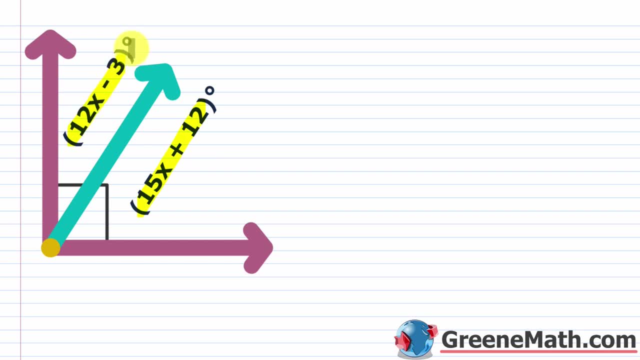 given by this guy right here, the 12x minus 3 degrees. So to find the measure of each angle here we use the fact that again, the complementary angles sum to 90 degrees. So I'm going to take this measure here, which is 15x plus 12.. I'm going to leave the degrees off for now, Then plus this: 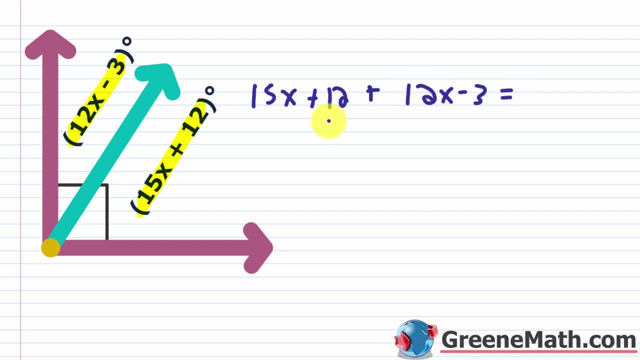 measure here, which is 12x minus 3.. I'm going to set this sum equal to 90 for 90 degrees, So we're going to solve this and basically 15x plus 12x is 27x. Then 12 minus 3 would be 9, and this equals. 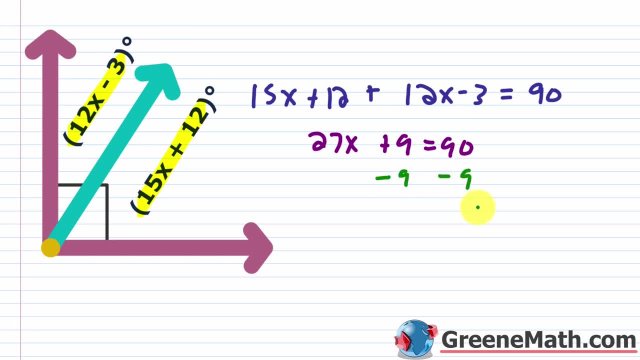 90. So what I'm going to do now is just subtract 9 away from each side of the equation, and of course this is going to cancel. We get 27x is equal to 81.. Divide both sides by 27, and you're going to. 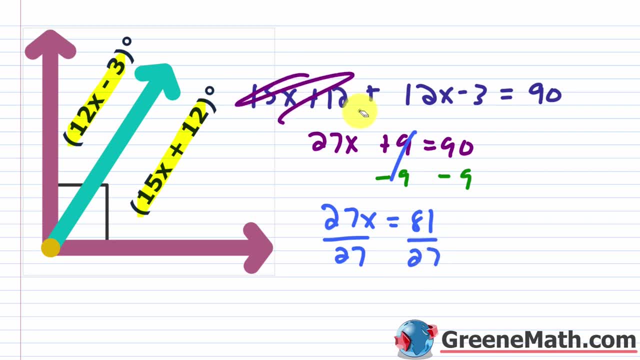 get that x is equal to 3.. So let me write that up here. We'll say that x is equal to 3.. So we're not done. We need to find the measure of each angle here. equals 3 just tells you what you need to plug in, So don't stop there. So we would have 15 times. 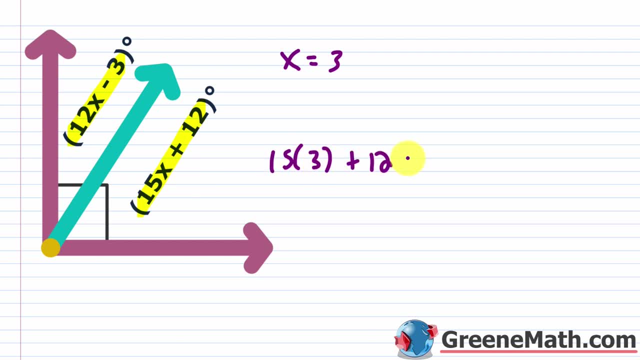 this 3 plus 12.. So 15 times 3 is 45.. 45 plus 12 is 57. So the measure here that you're looking for is 57 degrees. Then the other guy is going to be 12x minus 3.. So 12 times 3, and then minus 3.. 12. 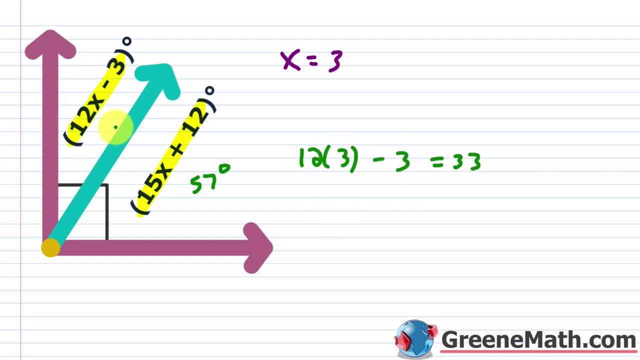 times 3 is 36.. 36 minus 3 is 33.. So the measure of this angle here is 33 degrees, And you can see that the measure of 57 degrees plus the measure of 33 degrees gives you a measure of 90. 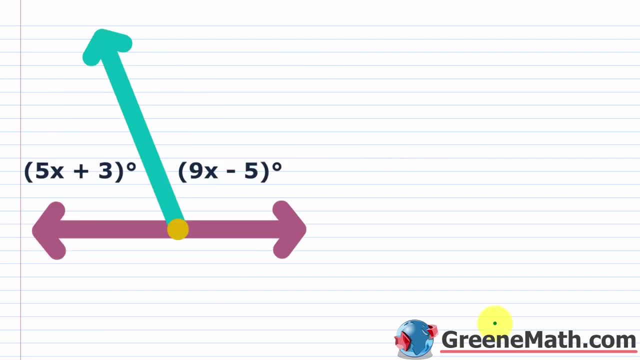 degrees, which again is the measure of the bigger angle. Okay, so now let's talk about supplementary angles. So we already know that a straight angle here. so if I started here and I rotated again, this is a half of a rotation. This forms a straight angle. It's 180 degrees. Okay, half of 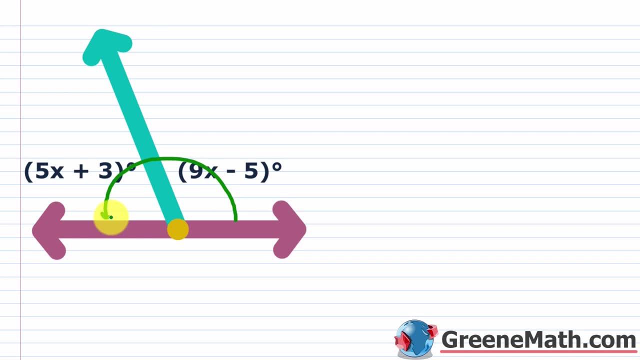 360 degrees, 180 degrees. That's how you remember your straight angle. So when the sum of the measures of two positive angles is 180 degrees, the angles are known as supplementary angles. So this example is basically the same in terms of. 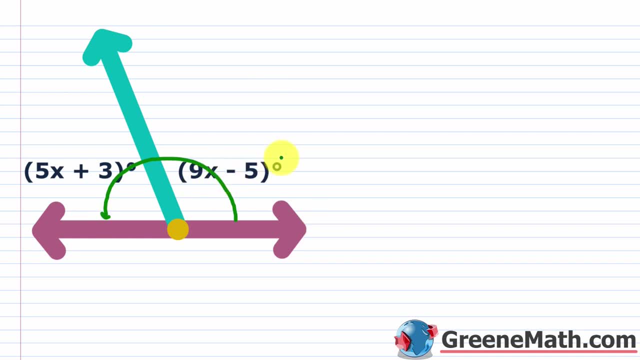 how you set things up. You have this angle here that's 9x minus 5 degrees, So 9x minus 5.. You have this angle over here which is 5x plus 3 degrees, So I just put those two as a sum, So 9x. 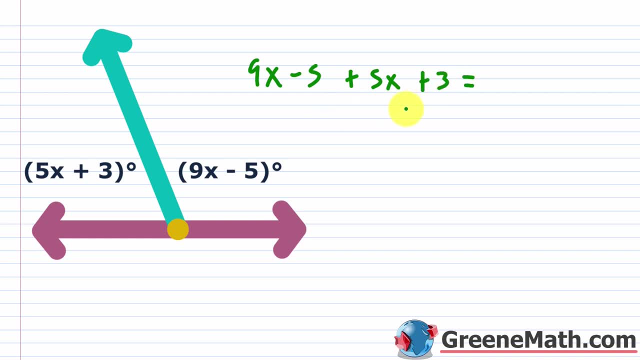 minus 5 plus 5x plus 3.. So I've got my sum going there And I set it equal to 180, 480 degrees. Again, that is the full angle, right, If I consider this all the way. 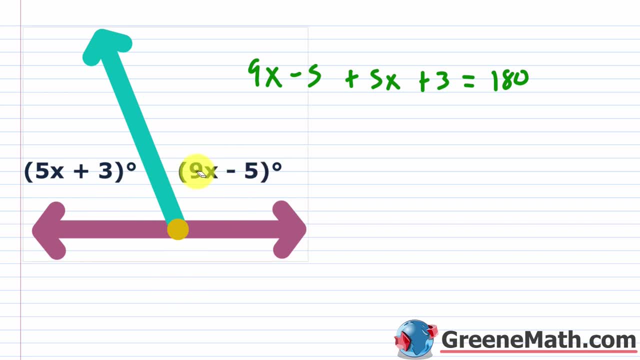 from here to here it's 180 degrees, And so what we do here is we just solve: 9x plus 5x is going to be 14x Negative. 5 plus 3 is, of course, negative 2.. So this equals 180.. Let's go ahead. 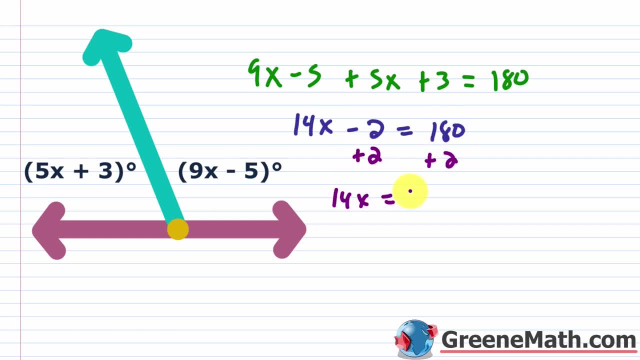 and add 2 to both sides of the equation, We get 14x is equal to 182.. We can divide both sides by 14 and find that x is equal to 13.. So x is 13.. Again, don't just put that in stop. You need to. 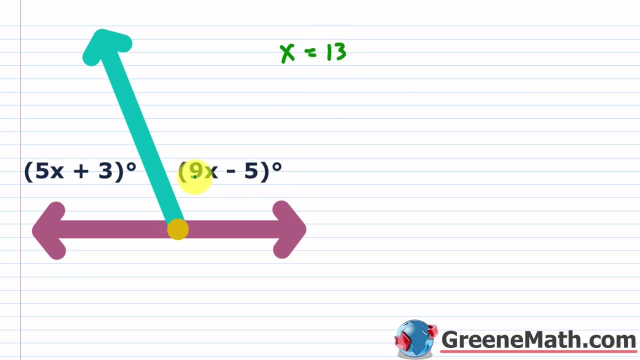 plug in to find out your measures. okay, So 9x 13,. 9x 13 minus 5.. 9x 13 is 117.. Minus 5 is 112.. So this guy is 112 degrees, okay, And then? 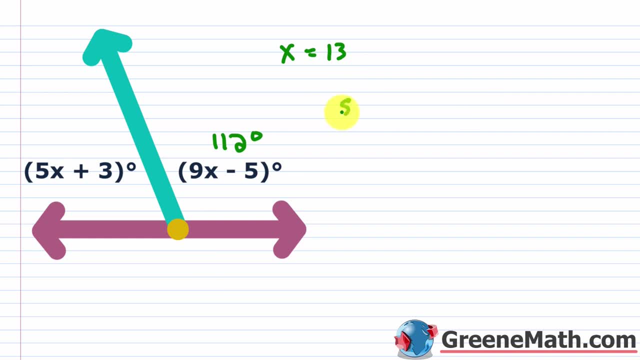 5x 13 is 65. Let me write that out. So 5x 13 is 65, plus 3 is going to be 68, okay, So this would be 68 degrees. So again, if you look at the sum of 68 degrees and 112 degrees, you get your 180. 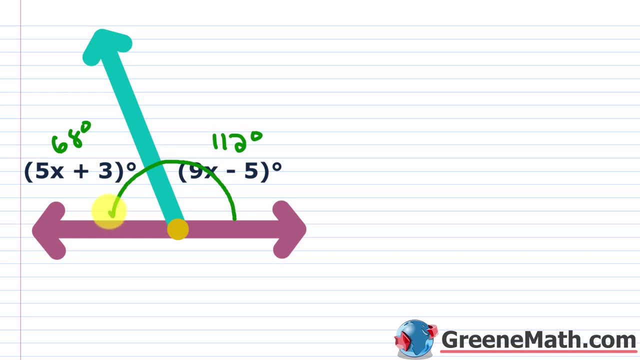 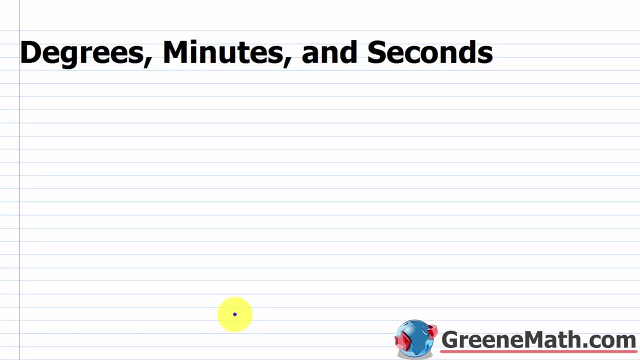 degrees, which, once again, is the total measure of this angle, right? So if we think about the whole angle, including this smaller angle and the other smaller angle, here's 180 degrees. So we would expect that 68 degrees plus 112 degrees to sum to 180 degrees, And in fact it does In this lesson we want to talk about 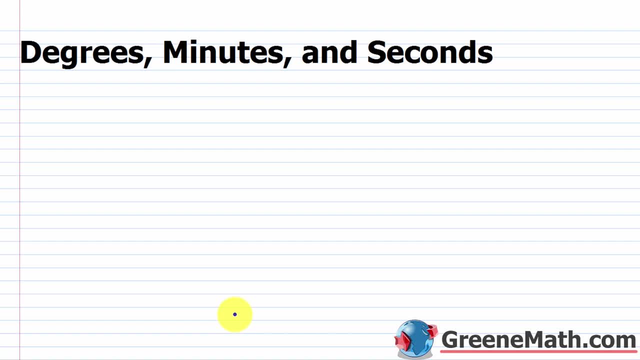 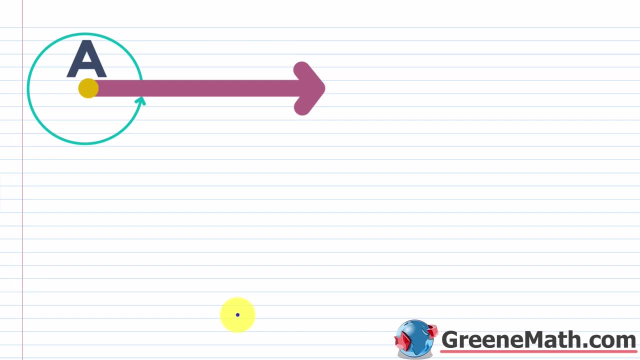 angle measures in degrees, minutes and seconds. All right. In our last lesson we talked about some of the basics that are involved with angles, And we also learned about the unit of measure known as the degree. It's how we can measure. 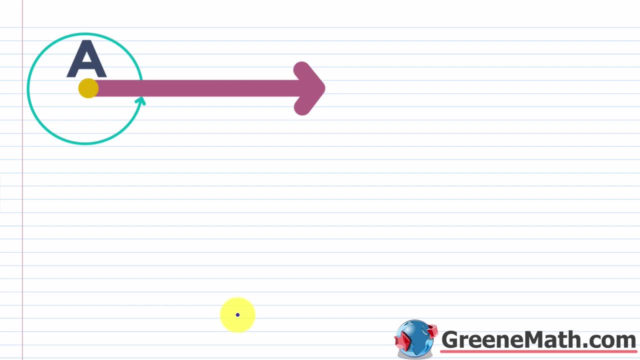 our angles. We also have radians, but we'll talk about that later on. So we learned that a complete rotation, or one complete rotation, is assigned the value of 360 degrees in terms of the measure of the angle that is produced. So let's say I started with two rays that were on top of each other. 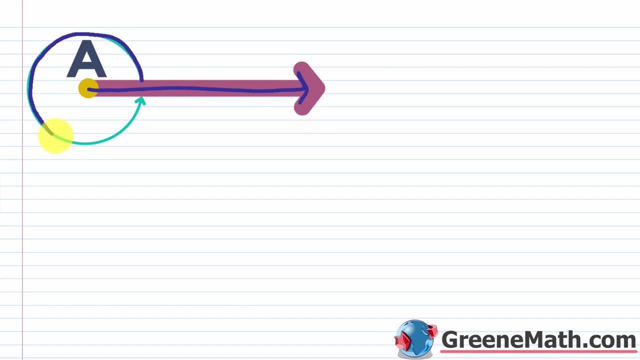 Again, I take this ray and I rotate it completely around. okay, Completely around. So what happens is the measure of that angle is assigned a value of 360 degrees. Now, if I think about this in terms of one over 360, so let's say I made that amount of a complete 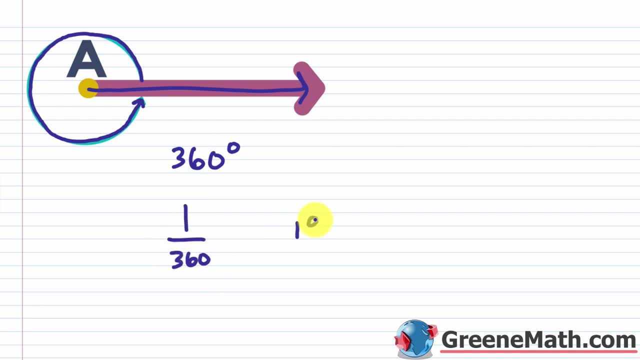 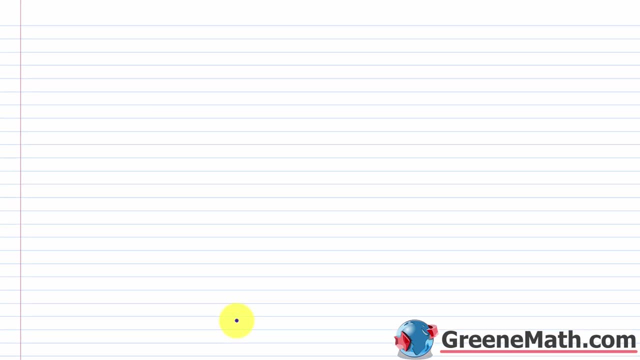 rotation. well, this is now going to be one degree. If I made five over 360, that amount of a complete rotation, that's five degrees, so on and so forth. Now, what happens when we need to measure an angle where the amount of the rotation is less than a degree? So it's a portion of a 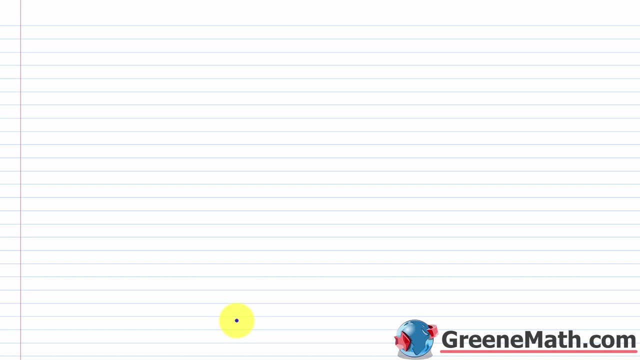 degree, a part of a degree, a fractional amount of a degree. Well, what we're going to turn to here is going to be minutes and seconds, So this is pretty easy to do. We're going to start with a fact: that if you have one degree and you divide it by 60,, this produces a unit known as the. 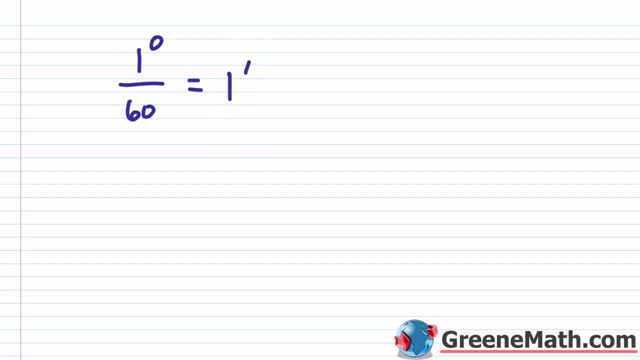 minute. okay, So this is going to give you one minute. So this is your notation for the minute. okay, Now you could also say that 60 minutes is going to give you one degree, right? So these two statements are saying the same thing. I can take one degree and divide it by 60 and get one minute. 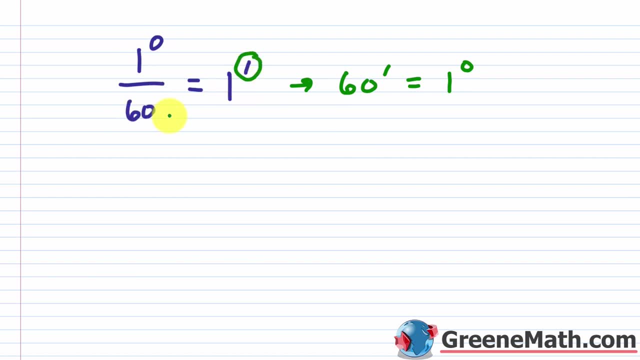 or if I multiplied both sides by 60, okay- and cleared the denominator, well, what I'd have is 60 minutes equals one degree, okay, So that's the same thing there. Now also we can go smaller, okay, So we can take. 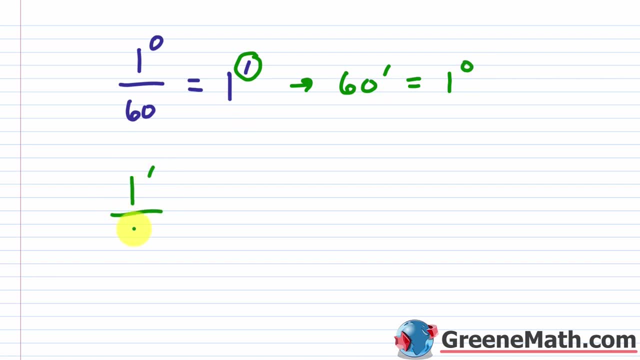 our minutes, so one minute, and we can now divide this by 60, and we're going to get a unit of measure known as the second. okay, So we're going to say one second like this, so that's going to be your notation for that, okay, And we can also again just multiply both sides by 60, and we can. 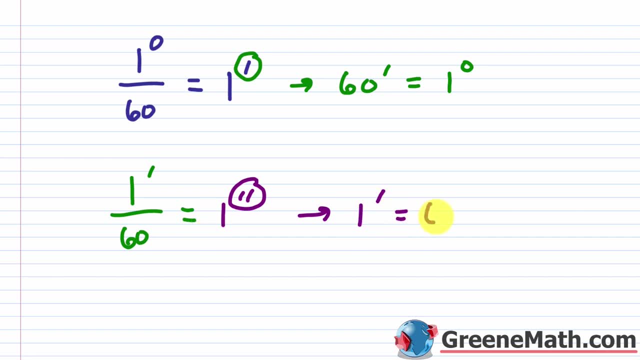 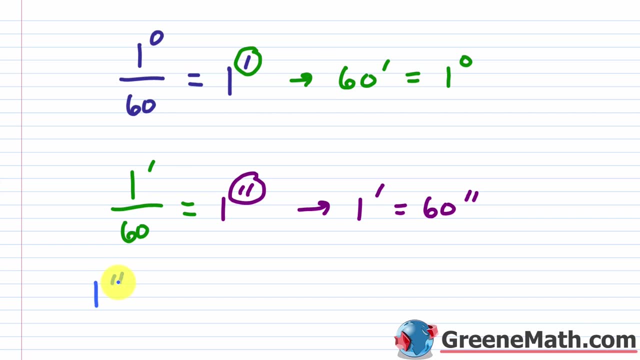 say that one minute is equal to 60 seconds, okay, So pretty easy to remember overall. Now, additionally, you can start with one second, okay, And you can say: this is equal to, again, one minute over 60, and this would be equal to what in terms of degrees? It would be one degree divided by 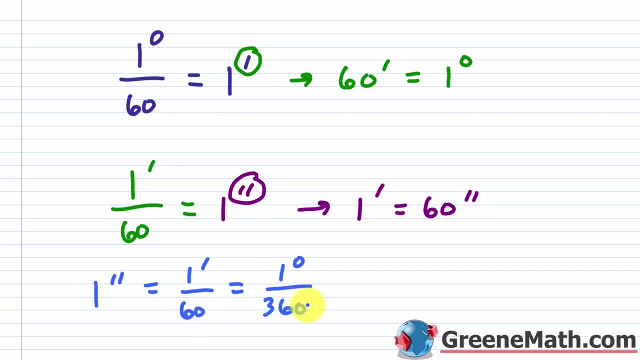 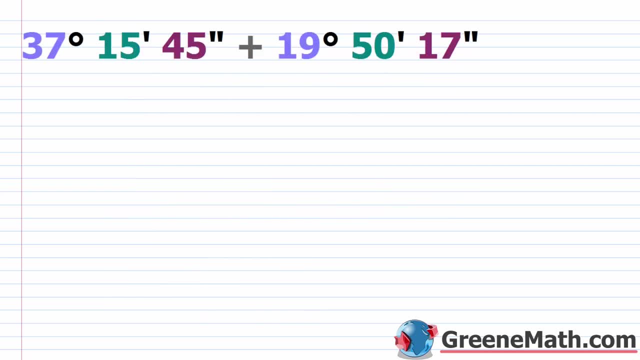 you're doing your homework, All right, let's go ahead and look at the first problem. We're just going to add two of these guys together. It's very simple. You just need to understand how the carrying process works. So let me explain. I'm just going to set this up vertically. You don't? 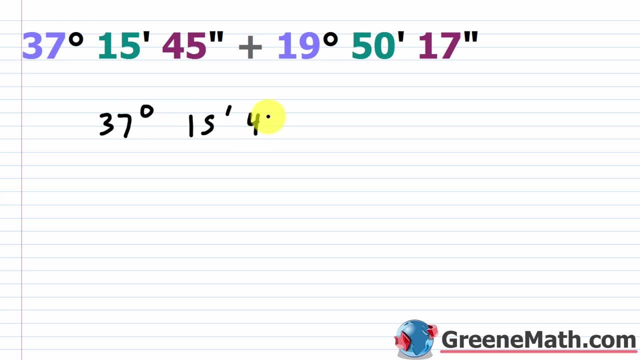 have to, but I think it's easier to do it that way. So let's just set this up vertically. So 19 degrees, we got 50, and we got 17 here. So what I have here is 37 degrees, 15 minutes. 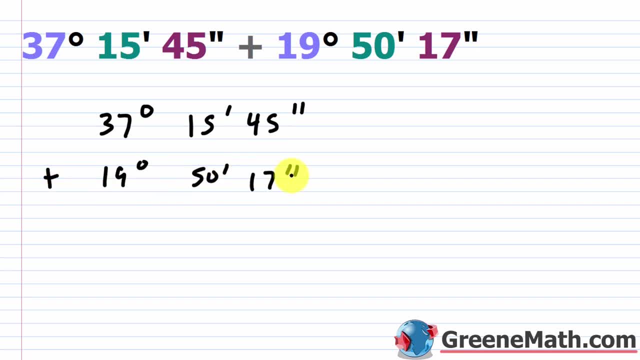 45 seconds plus 19 degrees: 50 minutes 17 seconds. Okay, so we're adding this together. So we know when we do a vertical addition, since we have a base 10 system, if you get a digit that is 10 or larger, you do a carrying process. Well, here, 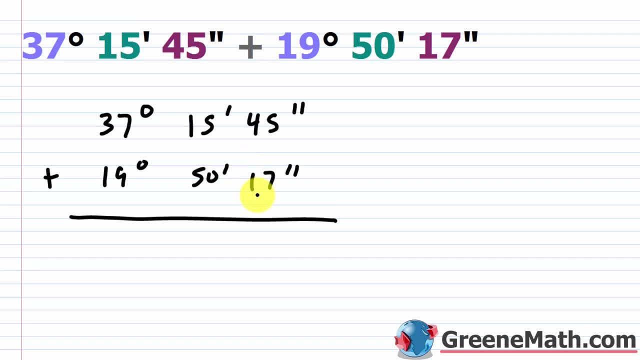 because of the way we convert things, we're looking for a value of 60 or larger to carry. So when I add 45 plus 17,, I get 62, right? So basically, this is saying that I have 62 seconds. 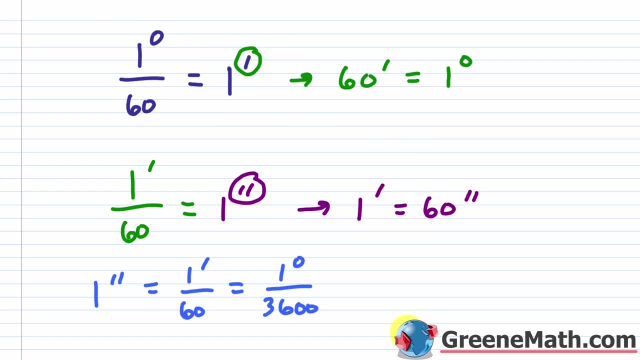 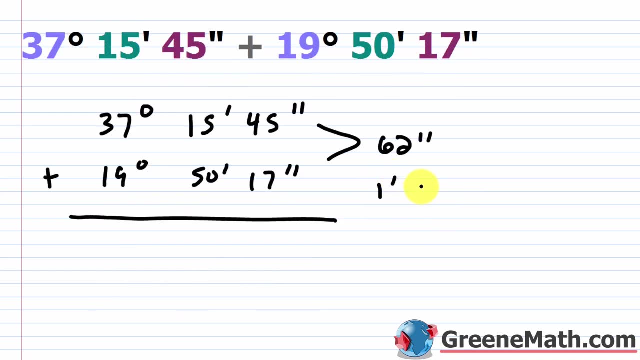 But again, if we go back up here, we know that 60 seconds equals one minute. So really, what I could say is that this is one minute and two seconds. right, So this is the carrying process you're going to use, You're. 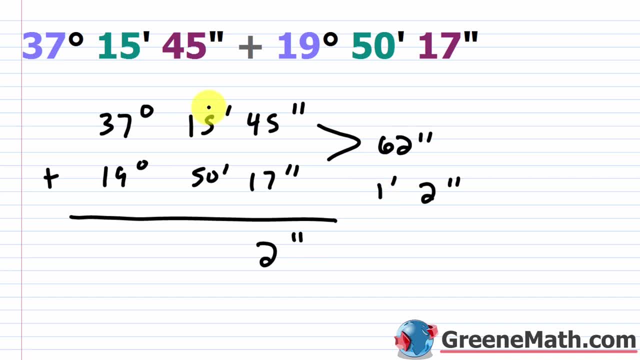 going to put two seconds down here and you're going to carry this one into the next column, okay, Just like if you were doing a vertical addition. it's no different, It's just you're changing the way you think about things because you're using 60 now. okay, So in this one, 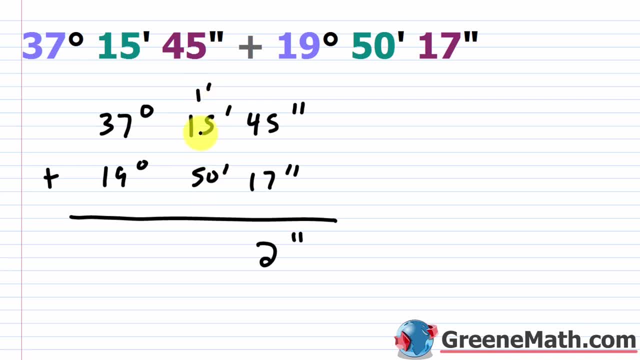 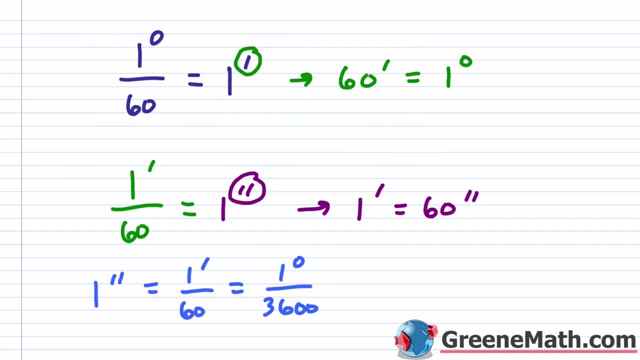 I've got 1 plus 15 plus 50. So 1 plus 15 is 60. So 1 plus 15 is 60. So 1 plus 15 is 60. So 16 plus 50 is 66. So again now we have 66 minutes And again, if we go back we know that. 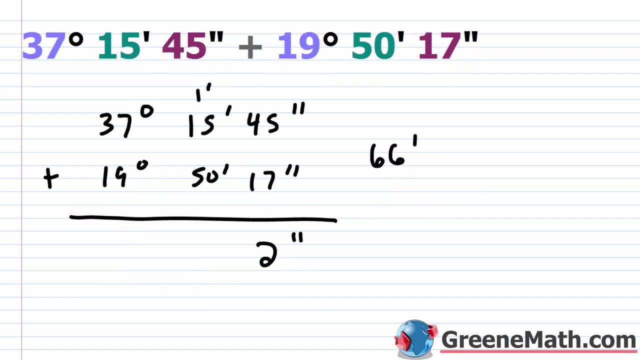 60 minutes equals one degree, So I can say that this is one degree and six minutes. okay. So I'm going to put my six minutes down here. I'm going to carry my one degree up and over to the next column And now I'm good to go. I do 1 plus 37,, which is 38,, and 38 plus 19,, which is going. 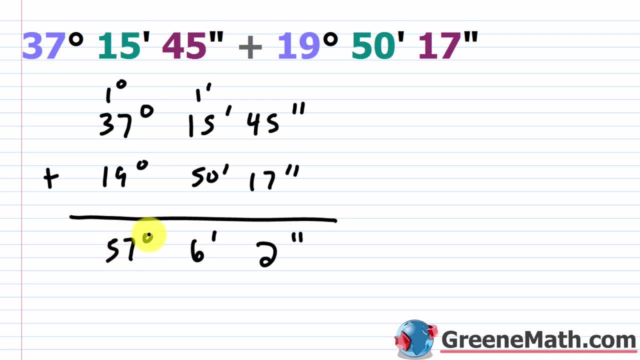 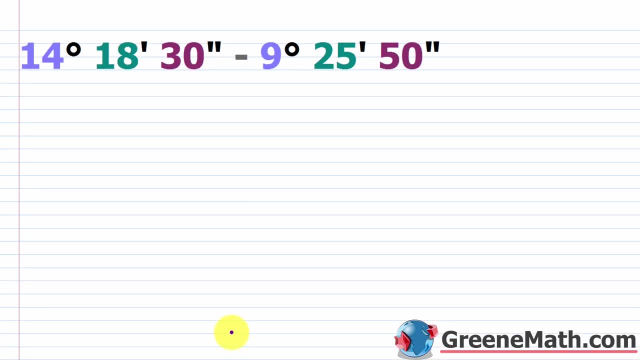 to give me 57.. So 57 degrees. So the answer here would be 57 degrees, six minutes and two seconds. All right, Now let's move on and talk about a subtraction problem. So you're going to find the process. 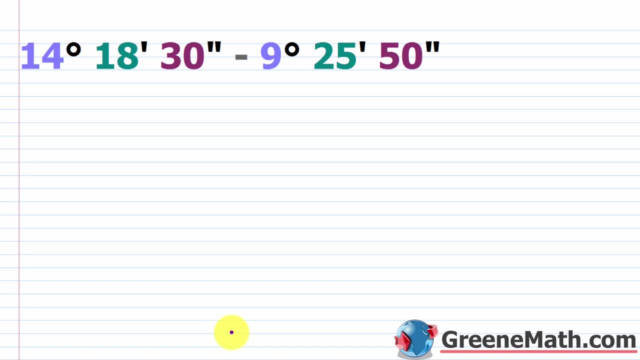 very similar to vertical subtraction, So let's just go ahead and set this up. So we have 14 here Degrees- 18 minutes 30 seconds. We have 9 degrees- 25 minutes 50 seconds. So put my: 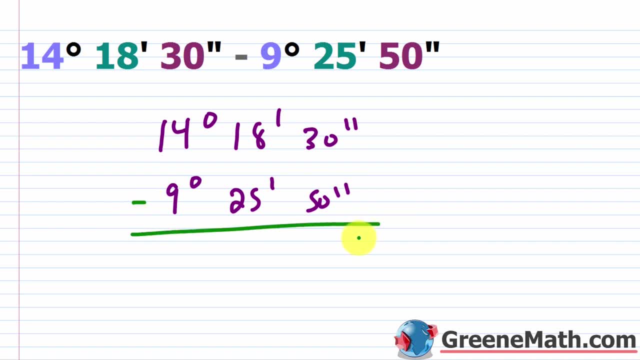 subtraction, sign out here, And what you're going to do is think about the fact that, again, I have 30,, I have 50. So I want to subtract here. So what I have to do is borrow right And think. 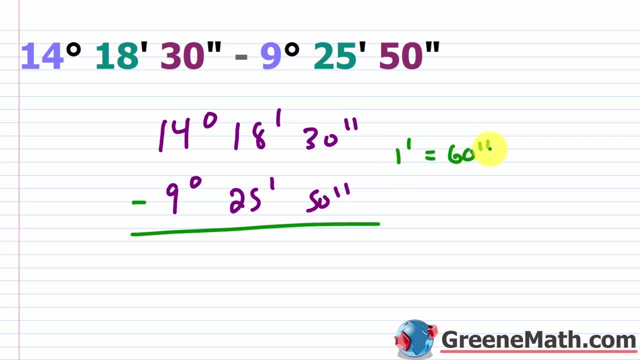 about the fact that one minute is equal to 60 seconds, right? So if I take one away from this and make this 17 minutes, now I can take this and convert it into seconds. So I can say: 30 seconds plus 60 seconds would be 90 seconds. So I'm just going to put 90 seconds there. I'm just borrowing. 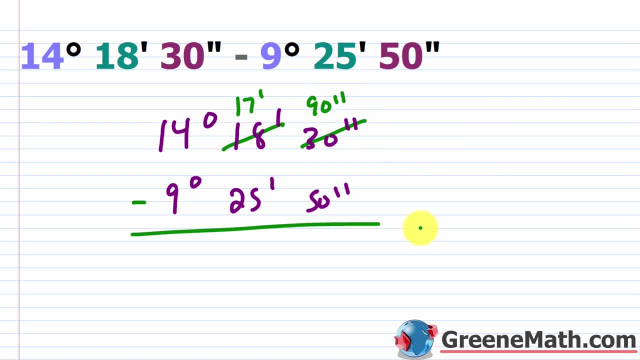 Again, just like I do with vertical subtraction, same thing. I've just got to get used to that number of 60,. okay, So 90 minus 50 is going to be 40. So this is 40 seconds. Then, when I get, 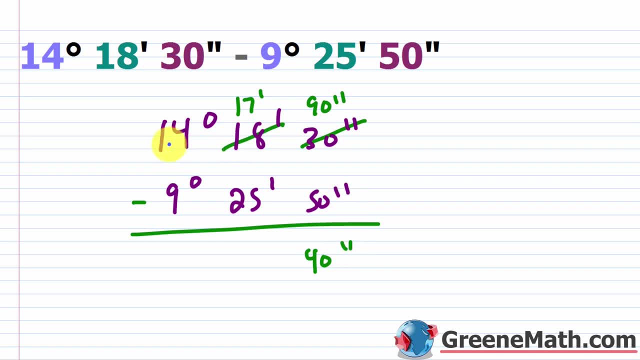 over to this column. here I've got to do the same thing again, So I've got to borrow. I'm going to borrow here and put this as a 13 degrees And remember: if I think about one degree, it's equal. 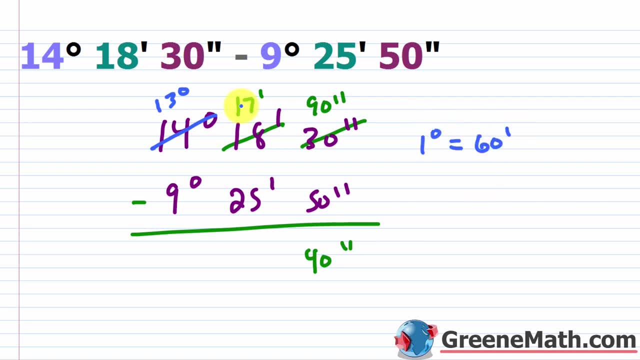 to 60,. okay, 60 minutes. So I'm going to add 60 to 17.. That's going to give me 77.. So 77 minutes And then 77 minutes minus 25 minutes is going to give me 52.. 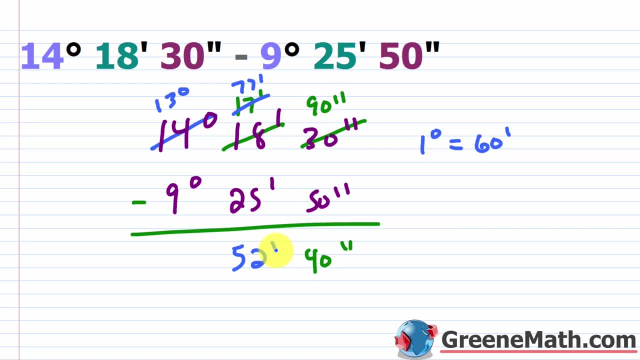 So now I move into my leftmost column. I have 13 degrees minus 9 degrees, That's just going to be 4 degrees. So my answer here will just be 4 degrees, 52 minutes and 40 seconds. Okay. 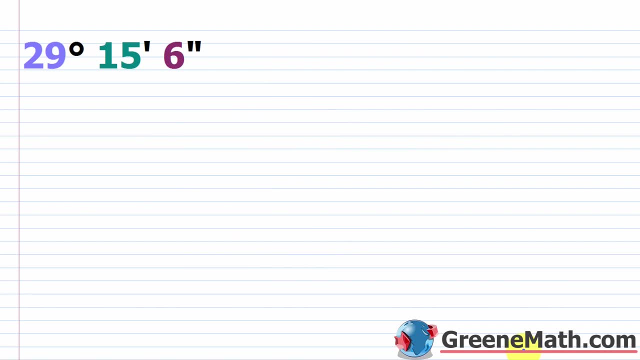 Let's find the complement and also let's find the supplement of the angle that's given. So we know that complementary angles sum to 90 degrees. We know that supplementary angles sum to 180 degrees. So if you're asked to find the complement of this angle, 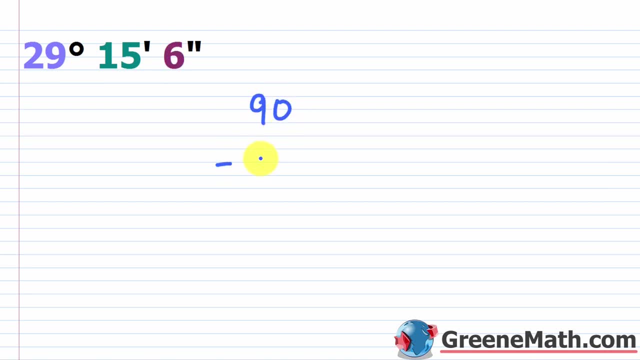 what I would do is I would say I'm going to do this, So I'm going to do this. I'm going to subtract 90, okay, minus this- 29 degrees, 15 minutes 6 seconds. So of course you need to. 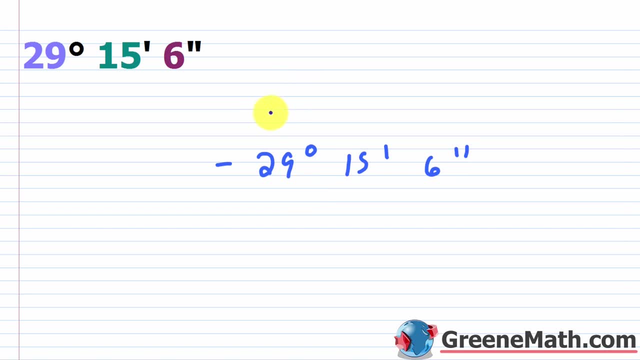 borrow here, So you can just go ahead and write this as 89 degrees, okay, And I'll put this as 60 minutes. You need to borrow again, So let's just write this as 59 minutes And let's just go ahead and write this as 60 seconds. So all I did was I took the 90,. 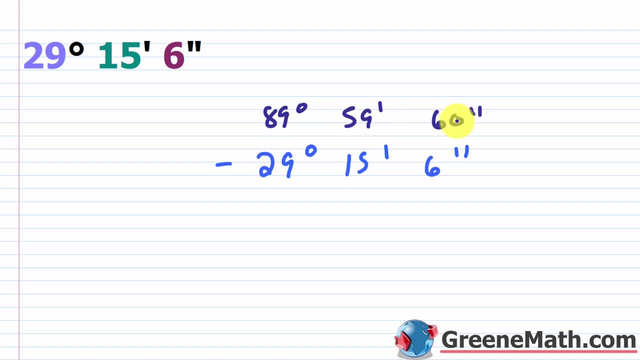 and I borrowed and I borrowed again So we can do our subtraction. okay, So we go through. Now we're good to go. 60 minus 6 is 54. So this is 54 seconds: 59 minus 15. 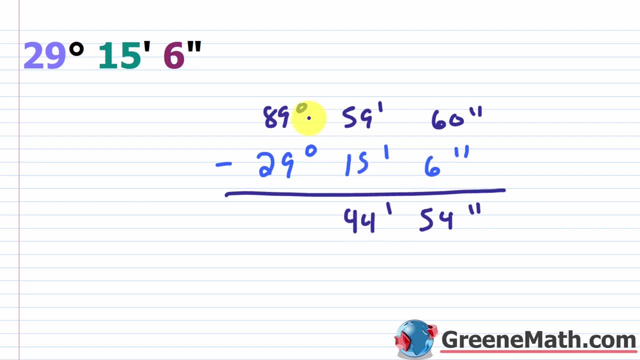 is 44. So this is 44 minutes, And then 89 minus 29 is going to be 60. So this is 60 degrees. So the complement of this angle here is going to be 60 degrees, 44 minutes, 54 seconds. Now. 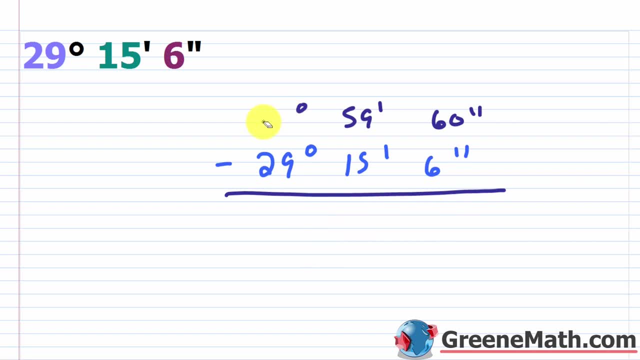 similarly, you can erase this part And up here, what I'm going to do is I'm going to put 179.. Nothing else will change, Because if I put 180 there again, I'd have to borrow and then borrow again. okay, So. 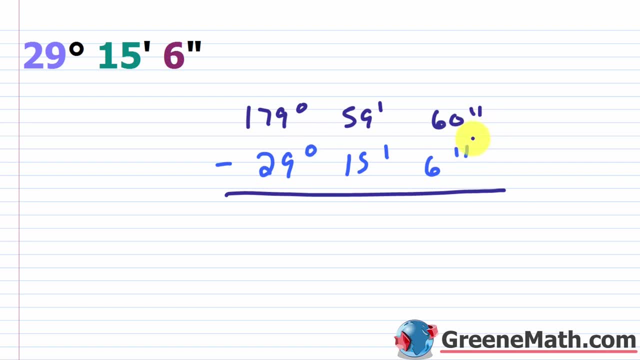 this is how you would set it up, And once you've done this, it's very easy. You just go through and say: okay, well, 60 minus 6, we know, that's 54. So 54 seconds, 59 minus 15, again, we know. 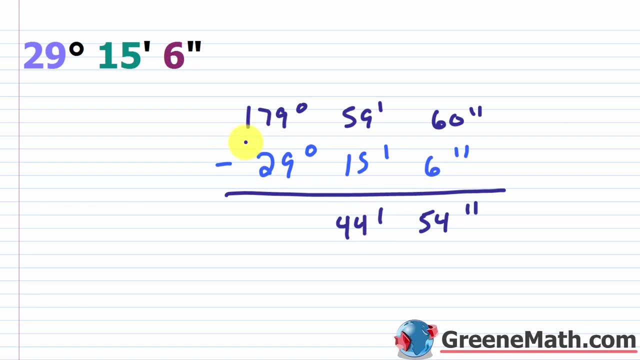 that's 44. So 44 minutes. And then 179 minus 29 is 150.. So 150 degrees there. So the supplement of this angle would be 150 degrees, 44 minutes, 54 seconds. All right, So now what we want to do. 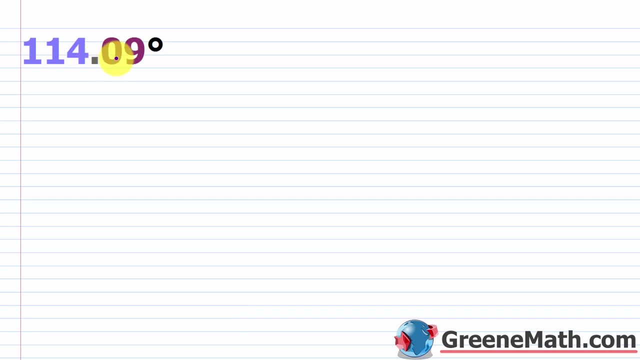 is go from this decimal form here, This 114.09 degrees, to degrees, minutes and seconds. So this is a pretty common task and very easy to do. So in the end, you want something that looks like this: You're going to have: 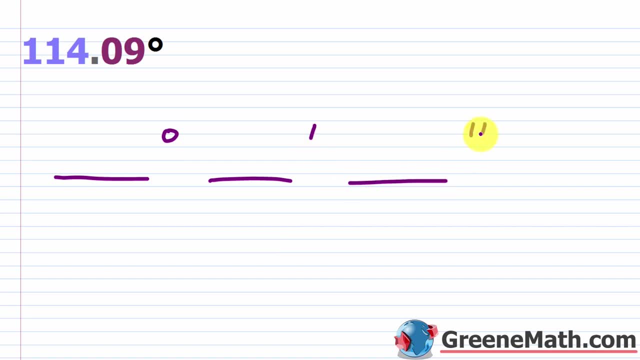 degrees. you're going to have minutes and you're going to have seconds. okay, So you take the part in front of the decimal point, the 114, that whole number part and just put it right here for your degree. okay, So it's 114 degrees. You're good to go with that. Now you move on to 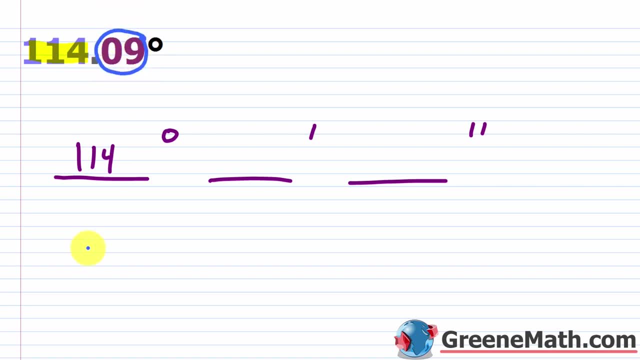 the part after the decimal point. So this part right here. you're going to go with that. Now point 0.09.. So .09 degrees is what I have left over after I fill that out. Now you want to. 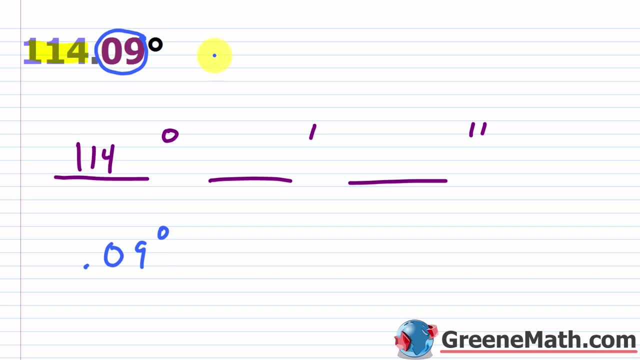 convert this into minutes first. okay, So remember, one degree is equal to 60 minutes. So to get this in terms of minutes, I need to multiply by 60, okay, So I would take this and let me just erase this. We don't need this. So, times 60, this would give me 5.4, okay, 5.4.. 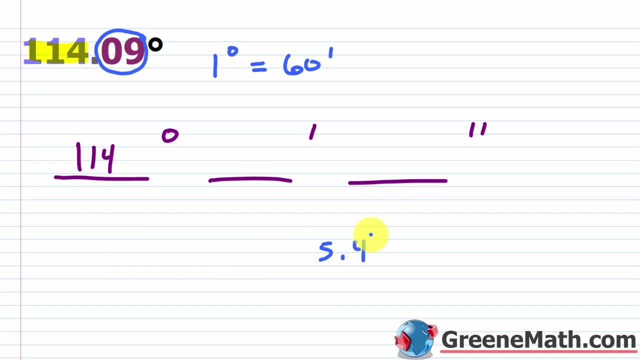 Now, this now is in terms of minutes. So this is in terms of minutes. I'm going to take the whole number part again and I'm going to just drag that up here. So I'm going to put 5 here and now I'm going to say that I have 0.4 minutes. 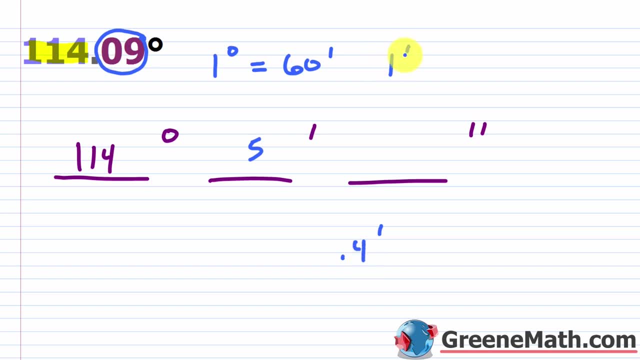 So remember, when you think about it you have: 1 minute is equal to 60 seconds. Okay, So I'm just going to multiply this now, this 0.4, by 60 to get it in terms of seconds, and this is going to give me a value of 24.. 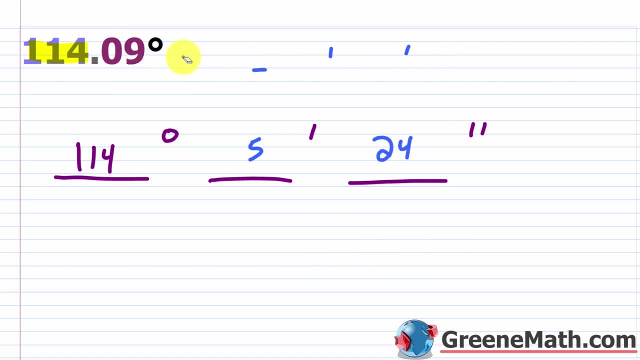 Okay, So when we convert this over, what we end up with is 114.09 degrees, is 114 degrees, 5 minutes 24 seconds, And if you have a TI-83 or a TI-84, it will actually do this conversion for you. 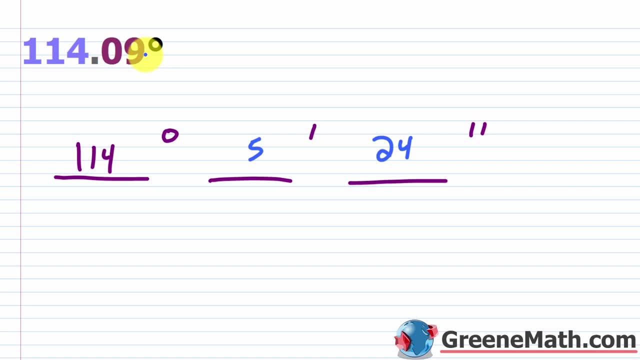 You want to type this number out first, Then you want to key up your angle button, which is usually second, and then angle, and you want to go down to the DMS for degrees, minutes and seconds, which is the number of seconds. 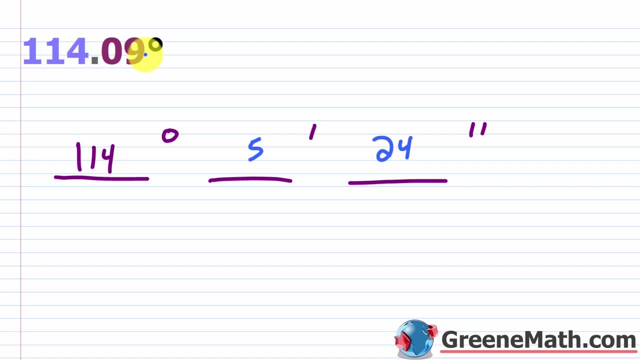 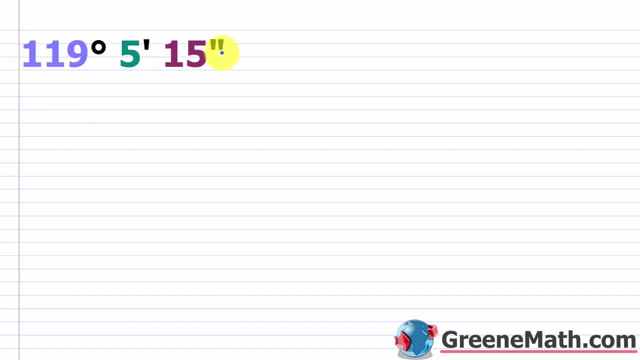 Okay, So when you hit that, it's going to give you this out as an output. Okay, So that's another way to do it. if you want to use your calculator, All right. So to wrap up the lesson, we want to look at this: 119 degrees, 5 minutes and 15 seconds. 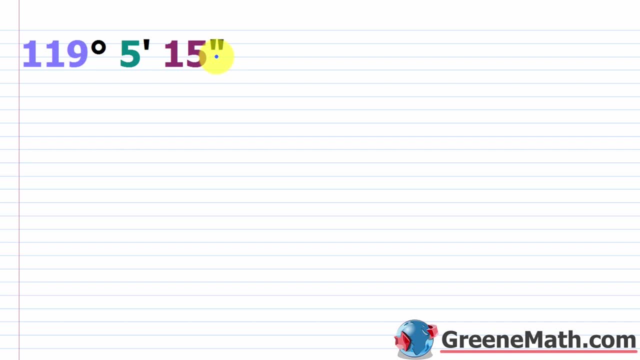 and we want to put this into a decimal form. So how can we do this? Well, we're going to start with this 119 here and then put a decimal point, And we want to think about the 5 minutes- how can we convert that? and the 15 seconds? 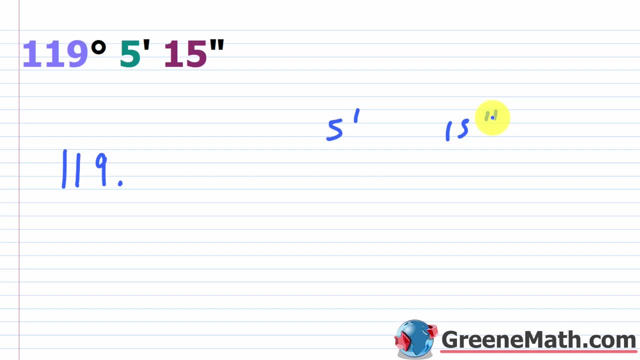 how can we convert that? Well, I want you to remember that the decimal point is the number of seconds, and I want you to remember that again. we think about it: 1 degree is equal to 60,. okay, 60 minutes. 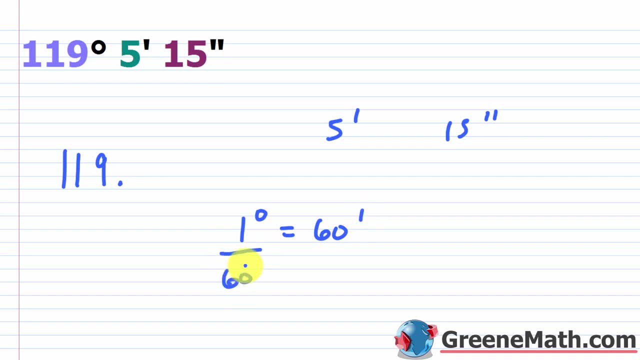 But also we said that 1 degree divided by 60 was equal to 1 minute. Okay, So if I have 5 minutes, okay, if I have 5 minutes, just think about the fact that that would be 5 degrees divided by 60.. 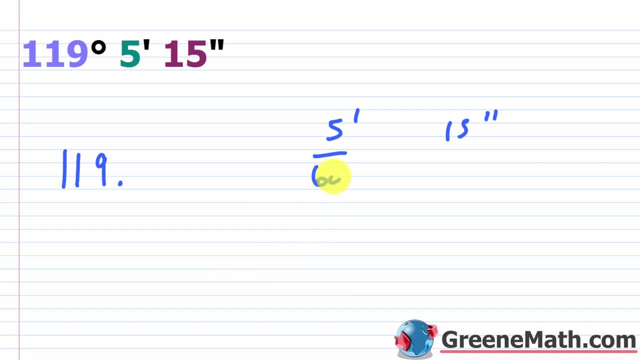 Okay, So I would say that I could divide this by 60,. okay, and I can get this in terms of degrees. Well, 5 divided by 60 is equal to 1 minute. 60 is going to be 1 over 12, but I'm going to reduce this in a minute because I'll talk. 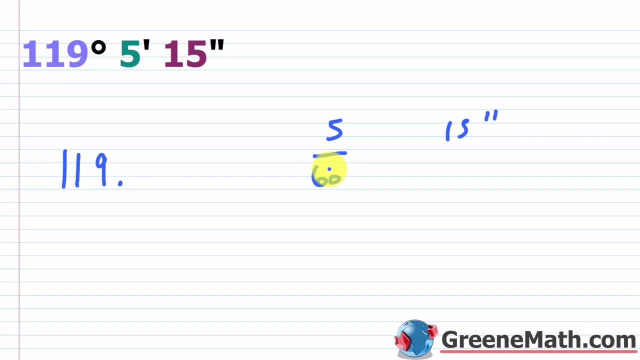 about this further. you're going to end up with this nasty repeating decimal, So just leave this alone for right now. All right, so to get this part in terms of degrees. remember, I told you in the beginning that, basically, if you had 1 second, okay, it was equal to 1 minute divided by 60.. 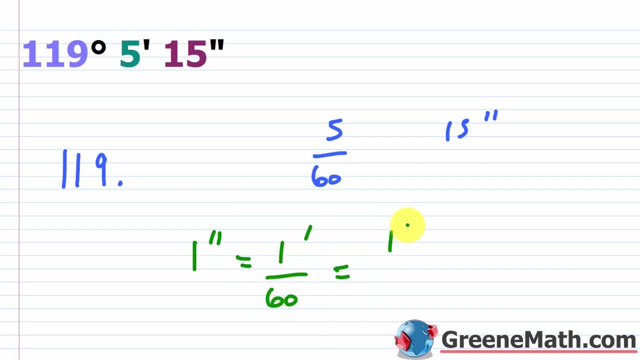 Okay, and 1 minute divided by 60, we could say is 1 degree divided by 3600.. Okay, So to get this in terms of degrees, we need to divide by 3600.. So let's erase this. So let's erase this and divide by 3600. 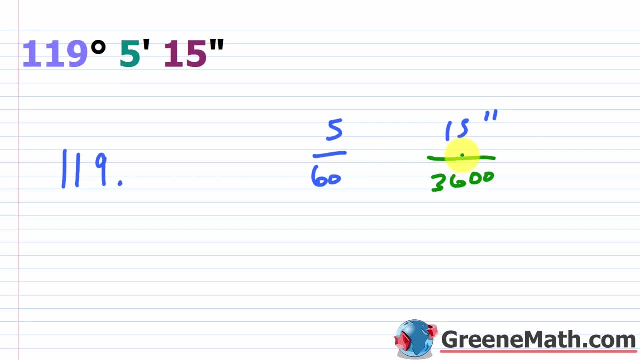 Okay, so at this point you would really be adding these two amounts together and basically, from those amounts you would get a decimal that you can put on here. Now, in a lot of cases, you're going to get a nasty repeating decimal for each of them. 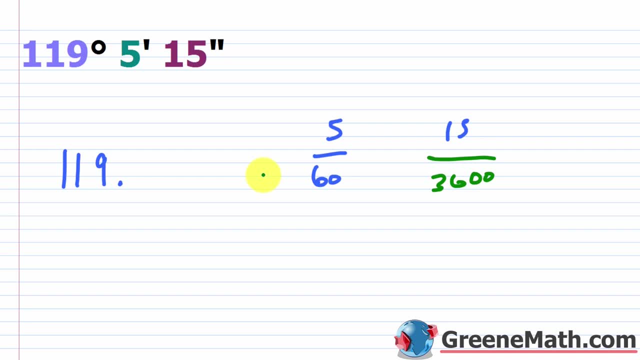 It doesn't happen all the time. Sometimes it works out nicely. But my suggestion to kind of limit that is to just get a couple of times and then you're going to get a common denominator going. So I'm just going to multiply this by 60 over 60.. 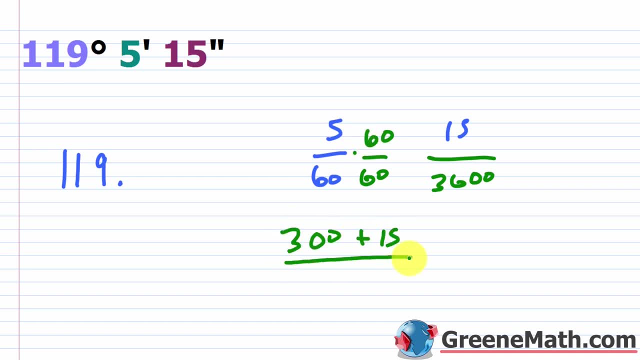 This is going to be 300 plus 15 over 3600.. And this is going to be 315 over 3600.. Okay, And this is going to work out to a nice decimal for us, which is .0875.. So .0875, and this is in terms of degrees. 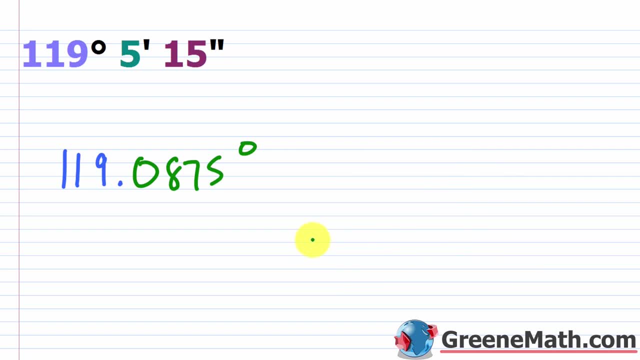 So not bad overall. just a lot of things to remember in terms of what the conversion is. Okay, Once you kind of have that memorized, it's very, very easy to do and a lot of times nowadays you can just do this on your calculator. 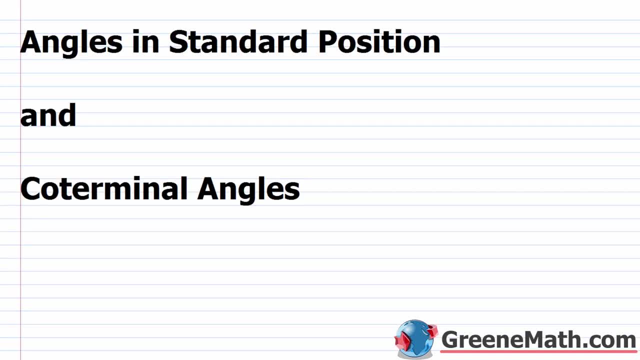 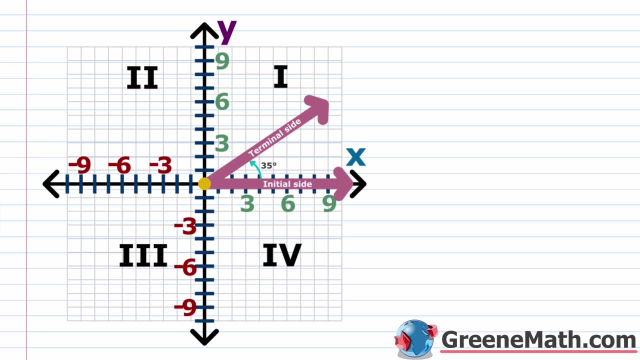 In this lesson we want to talk about angles in standard position and also we want to talk about coterminal angles. All right, so an angle is in what we call standard position if its vertex is at the origin and its initial side lies on the positive x-axis. 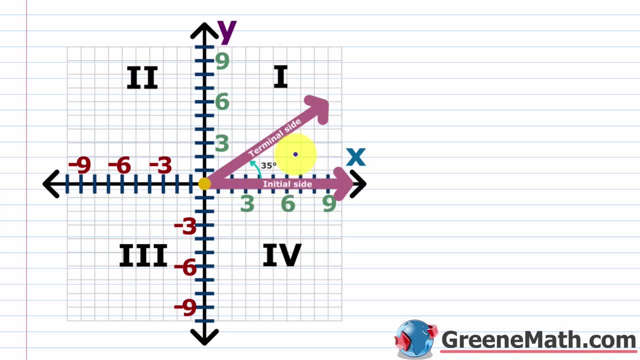 So that's all it is. That's the whole definition. So in this example here, you see, we have a little 35-degree angle And we can see that our vertex is at the origin okay, and we can see our initial side is on. 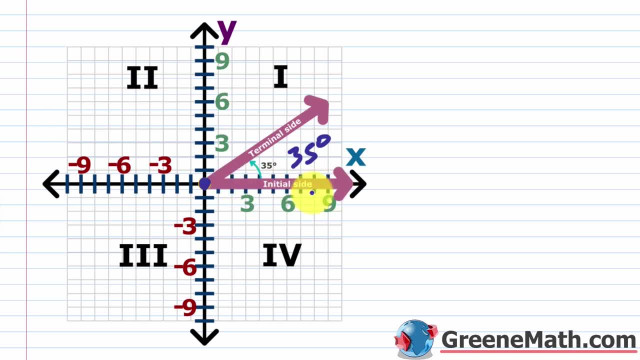 the positive x-axis, So this guy is in standard position. Now, additionally, when we have an angle that's in what we call standard position, it's said to lie in the quadrant where the terminal side lies. So in this case, my terminal side lies in quadrant one, okay. 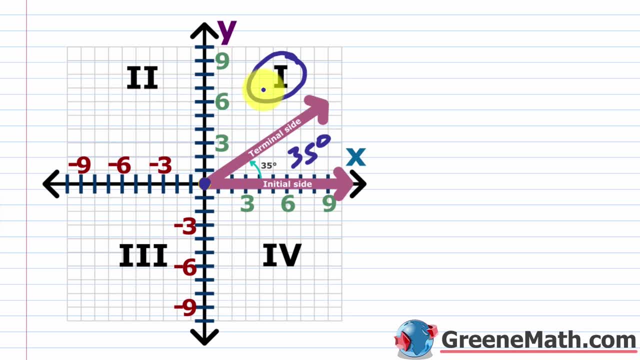 So this guy would lie in quadrant one. Now, additionally, you remember that these guys go counterclockwise, So this is quadrant two. Okay, So if you had an obtuse angle, you'd be in quadrant two. If you had an angle that was greater than 180 degrees, but less than 270 degrees, you'd 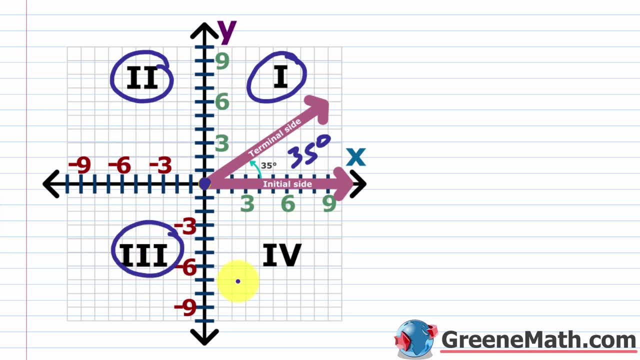 be in quadrant three, And then, if you had one that was greater than 270 degrees and less than 360 degrees, you'd be in quadrant four. Okay, Now something to keep in mind. you might get an angle whose measure is some multiple. 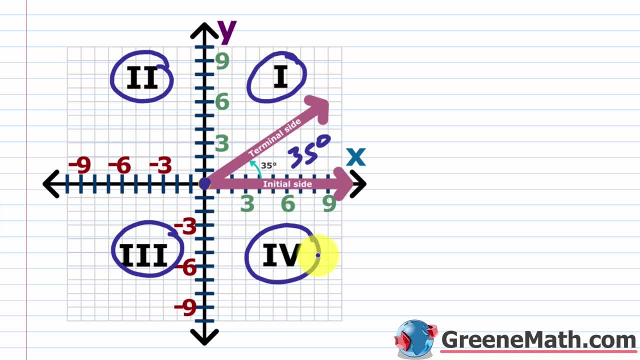 of 90 degrees. So it could be 90 degrees, 180 degrees, 270 degrees, 360 degrees, you know, so on and so forth. Well, in this case we have something known as a quadrantal angle. Okay, 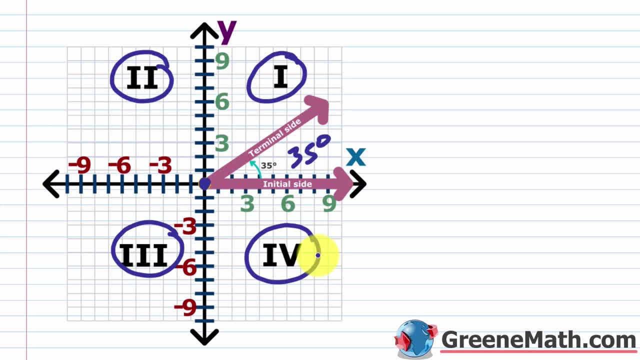 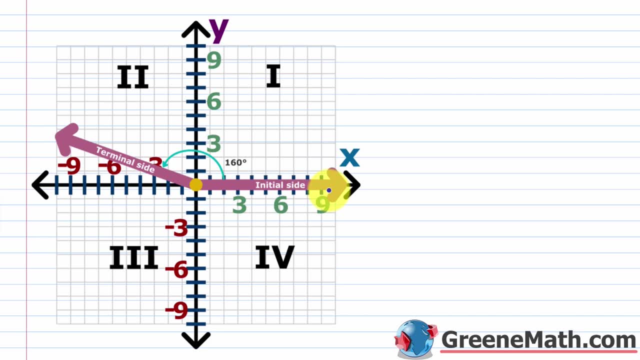 So you will not be in any quadrant. Okay, So that might be a question for you on your test. So another little quick example of this. we have another angle that's going to be in standard position. So again, the vertex at the origin, the initial side, is on the positive x-axis. 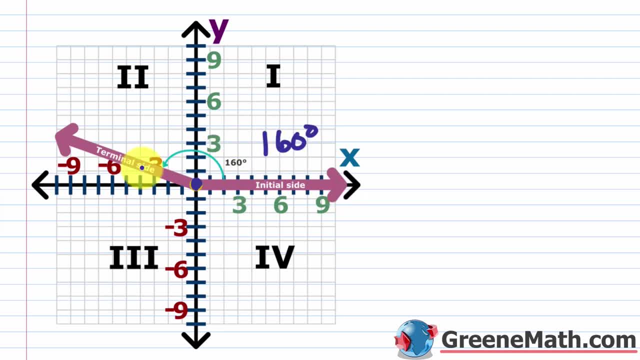 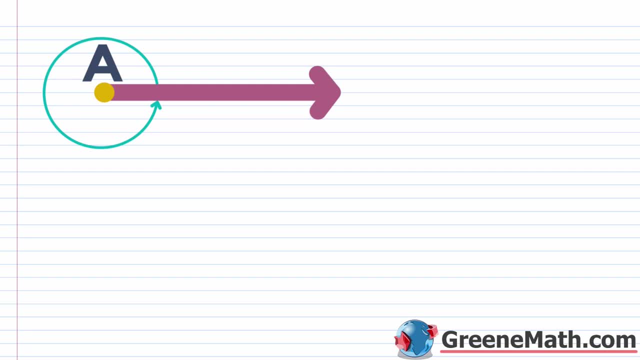 This guy is a 160 degree angle, So it's an obtuse angle and it's going to lie in quadrant two right, Because that's where its terminal side is Okay. So let's talk a little bit about getting an angle measure that's larger than 360 degrees. 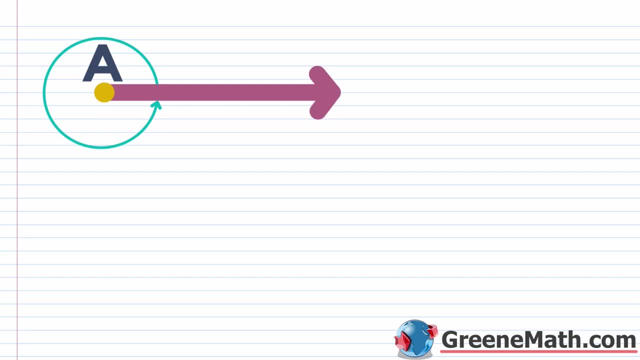 Okay So let's talk a little bit about getting an angle measure that's larger than 360 degrees. Okay So, let's talk a little bit about getting an angle measure that's larger than 360 degrees. We already know that the complete rotation, or one complete rotation of a ray represents 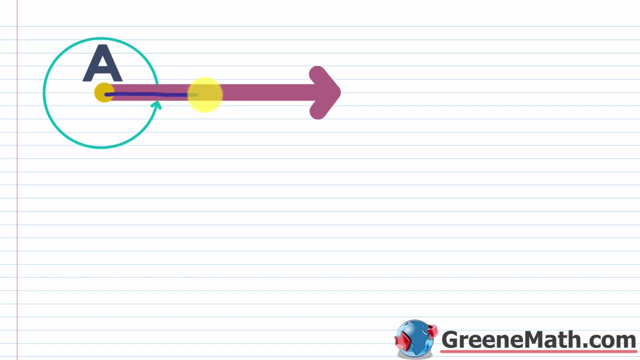 an angle whose measure is 360 degrees. So we've seen this in pretty much every video at this point. So we have two rays on top of each other If I rotate this guy completely around, so one complete rotation. that angle measures 360 degrees. 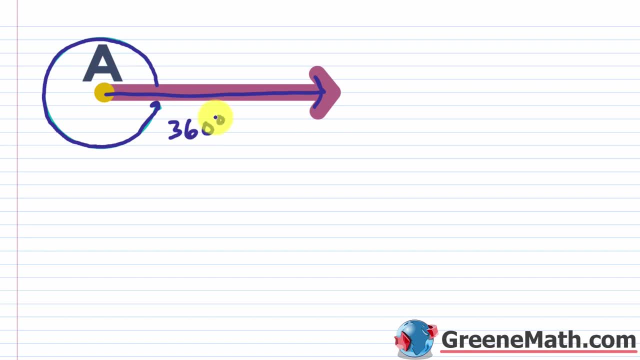 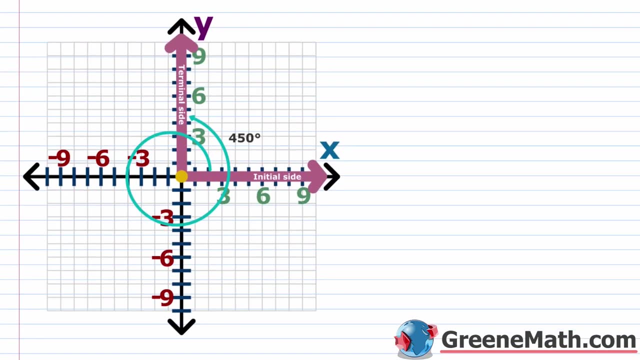 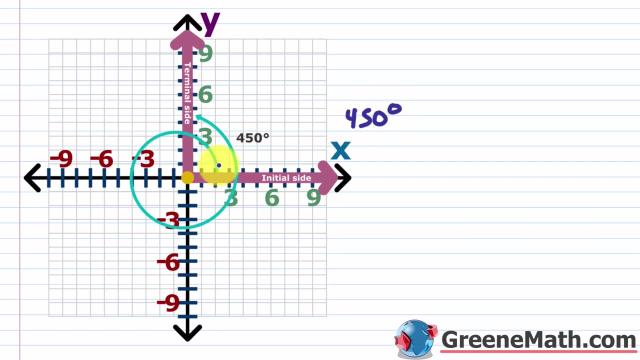 And let me put 360 degrees there And basically, if we keep going, we can generate angle measures that are greater than 360 degrees. So, as an example, here you can see that we have a 450 degree angle. So a 450 degree angle and we generate this by making one complete rotation. 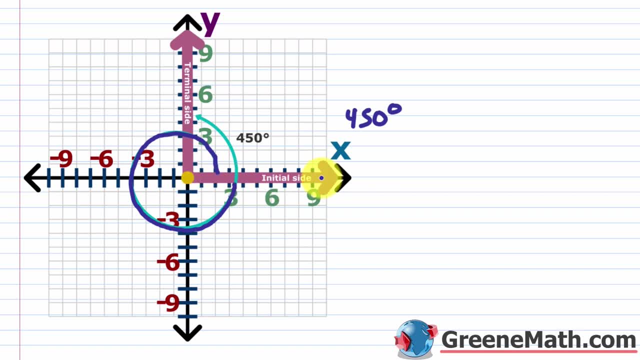 So one complete rotation. so to right there, okay, where the terminal side would be on top of the initial side, And then we keep going another 90 degrees. So you'll notice how this looks like a right angle or a 90 degree angle. 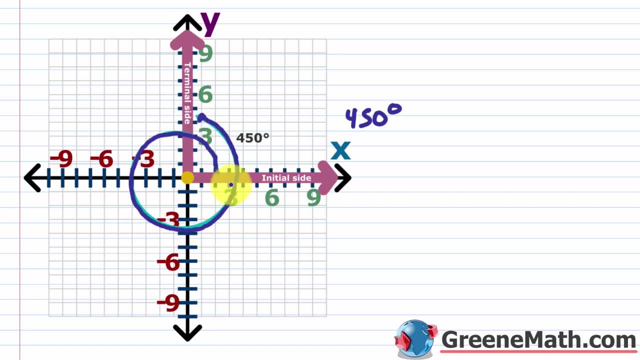 But basically we show here that we made one full rotation, plus we went another 90 degrees, So we get this 450 degrees. we take the 360 degree angle again from one complete rotation and we add to that 90 degrees. 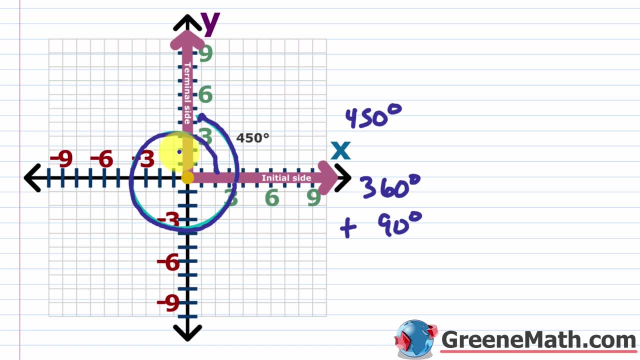 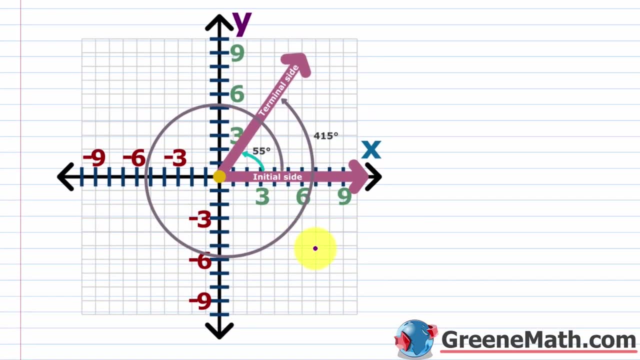 We know, from here to here is 90 degrees, because this is a right angle, And so we add those two amounts together and we get 450 degrees. okay, so that's where this guy comes from. All right, so now let's talk about these coterminal angles. 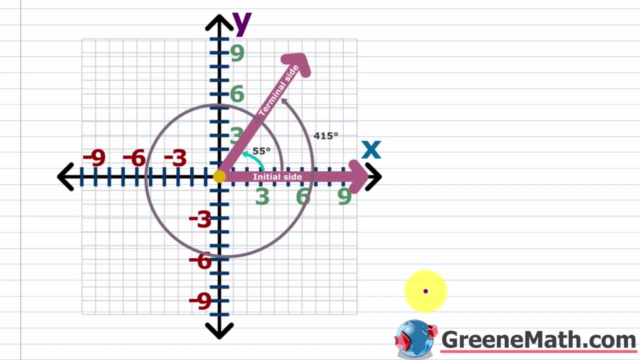 So the concept here is that coterminal angles are going to be angles that have the same initial side and also the same terminal side, but differ by amounts of rotation. The measures are going to be different by some multiple of 360, okay, and I'll show. 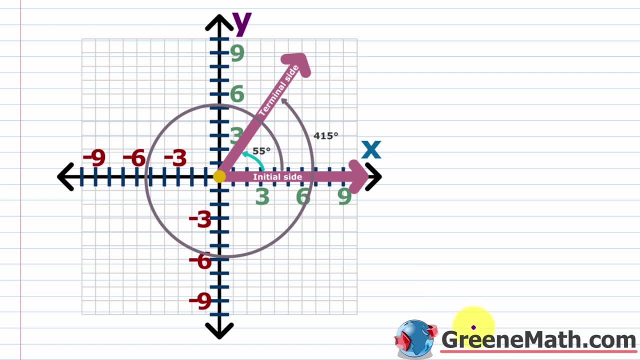 you how to calculate that in a moment. But basically, if we look at this first example, you see that you have a 55 degree angle and you have a 415 degree angle. So the same initial side, the same terminal side. 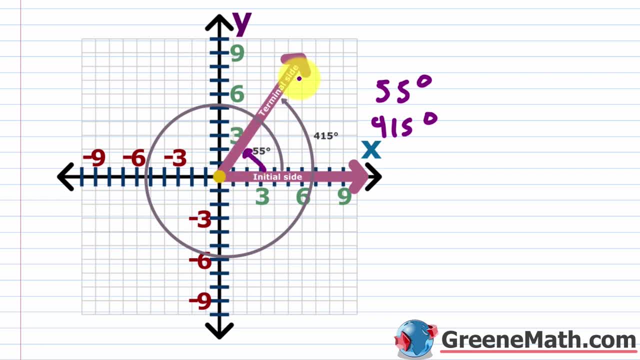 To get this first 55 degree angle, we start here and we just rotate here. that's all we do. But to get the 415 degree angle again, you're going to make more than one complete rotation. So you're going to go around once. okay, so that's 360 degrees. 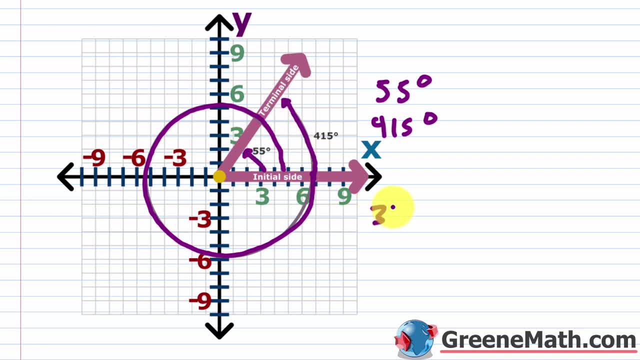 And then plus another 50 degrees. So in other words, you took 360 plus your 55, okay, let me put my degree symbol in each case, and this gives us the 415 degrees that we see from that angle. Now, to show this, without making a little diagram or a little graph, what you could. 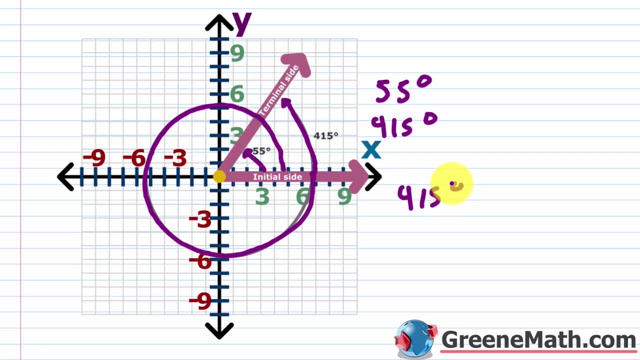 do is just subtract. Okay, so you can either do 415 degrees minus 55 degrees, and that would give you 360 degrees, or you could go the other way. Okay, it's going to be negative, but it doesn't matter. 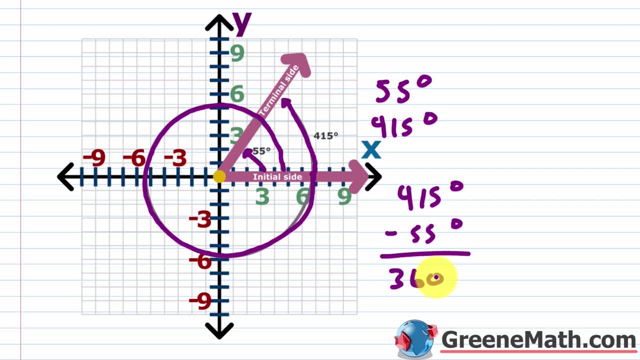 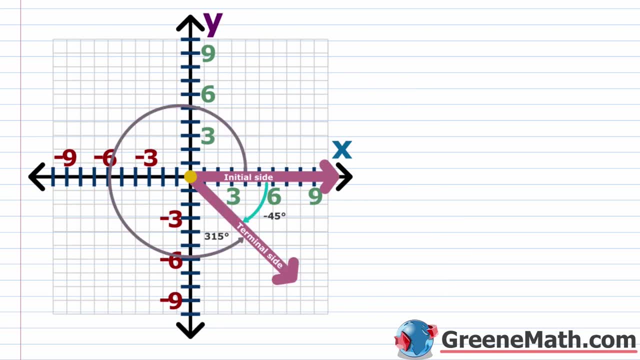 You're looking for some multiple of 360.. Okay, so if you did 55 degrees minus 415 degrees, you would get negative 360 degrees. Now let's look at another example of this. In this case you have one positive angle and one negative angle. 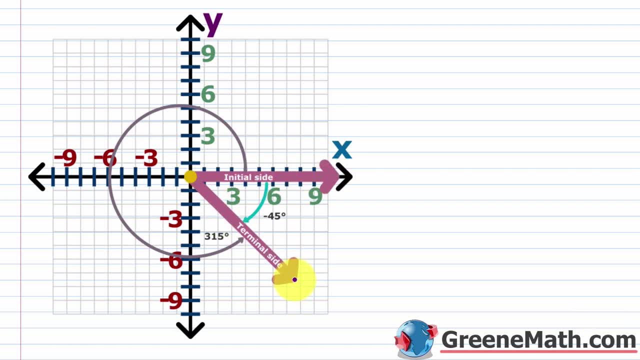 So this works as well. You have the same initial side and the same terminal side. So this guy is a negative 45 degree angle and this guy is a 315 degree angle. So we start here and we go again. if you're going clockwise it's a negative angle. 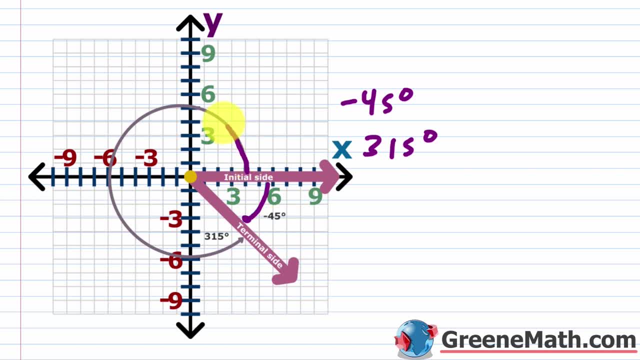 So this is a negative 45 degrees. Again, we're going counterclockwise, so it's positive and we go in this direction. So we're going around and this becomes 315 degrees. okay, If you were to subtract the 315 minus a negative 45, so 315 degrees minus a negative 45 degrees. 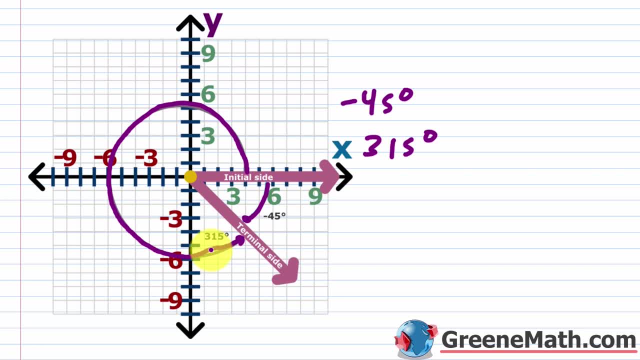 remember, minus a negative is plus a positive, you would get 360 degrees. If you were to subtract negative 45 degrees minus 315 degrees, you would get negative 360 degrees. So again, the way that you subtract is not going to work. 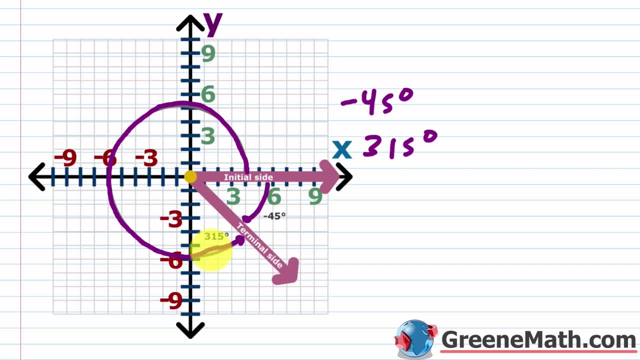 Okay, You're just looking for some multiple of 360 degrees to determine if these guys are cotermal. Again, same initial side, same terminal side. They're going to differ by some multiple of 360 degrees, That's all it is. 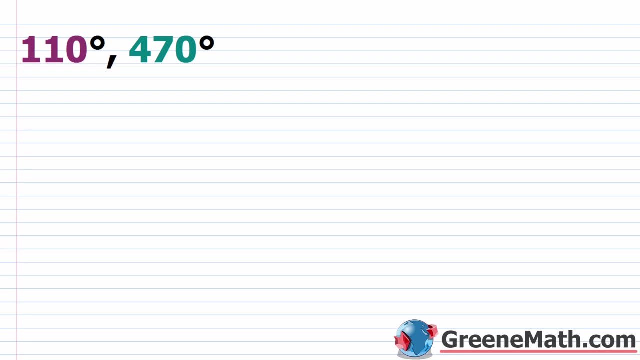 Let's look at the first example. So we have 110 degrees and 470 degrees. A lot of you can eyeball that and see that the difference between those two would either be: if you did 470 degrees minus 110 degrees, obviously that would be positive 360 degrees. 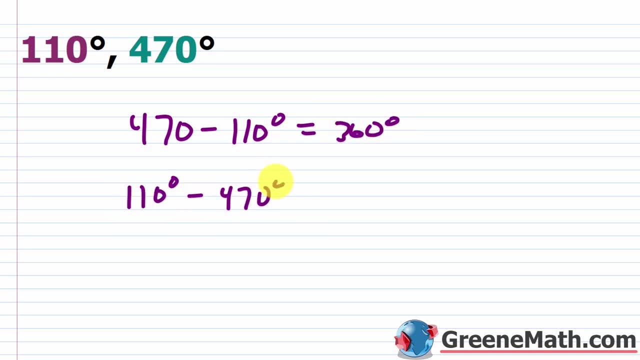 And if you did 110 degrees, you would get negative 360 degrees. Okay, If you did 470 degrees minus 470 degrees, that would be negative 360 degrees. But again, you're just looking for some multiple of 360 degrees. 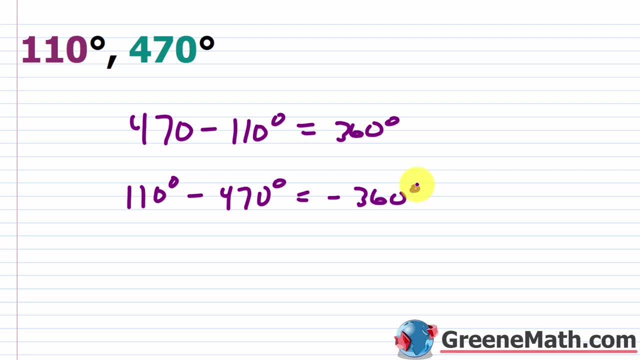 It could be positive or negative, it doesn't matter. Some multiple of 360 degrees. So in this case, we know these guys are cotermal. Okay, For the next one, we have 135 degrees and we have negative 495 degrees. 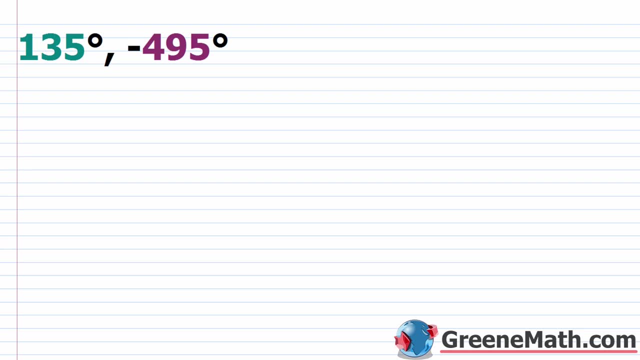 So again, you can just subtract. You could do 135 degrees minus a negative 495 degrees, which would be 135 degrees plus 495 degrees. In this case, that would give you 630 degrees. Okay, And if you don't know off the top of your head if that's going to be a multiple of 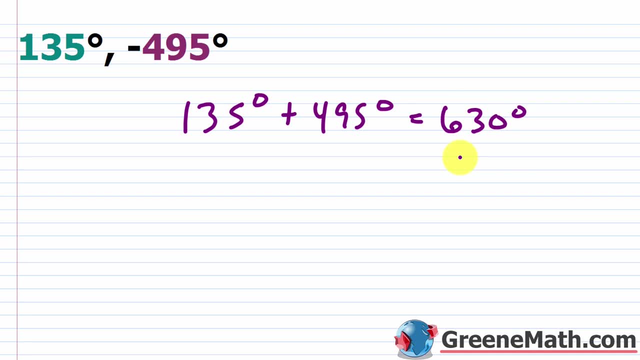 360 degrees. you just divide by 360 and see if you get a remainder. So if I punch that up on my calculator, I get 1.75.. So to say you don't have a remainder. remember you want something that's either a whole number, 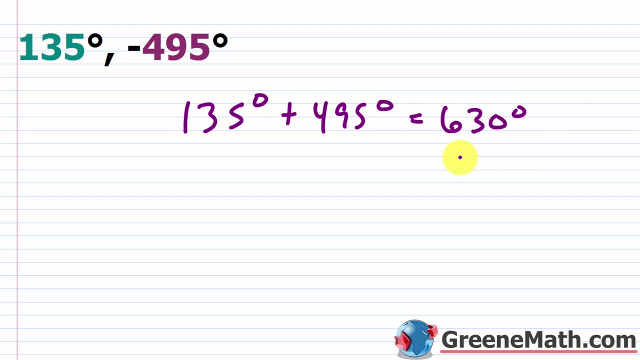 or an integer, right? You don't want a decimal part or a fraction or something like that, right? You want a whole number or an integer. So, because we have 1.75, we know that 630 is not divisible by 360.. 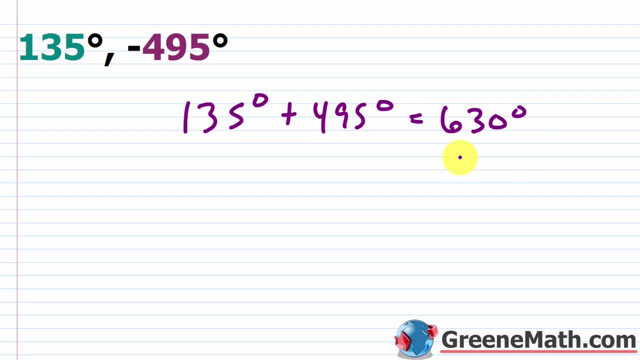 So this guy is not some multiple of 360, so these guys are not coterminal angles. All right, For the next one, we have 335 degrees and 2,135 degrees. So again, you could just subtract. You can subtract in any order. 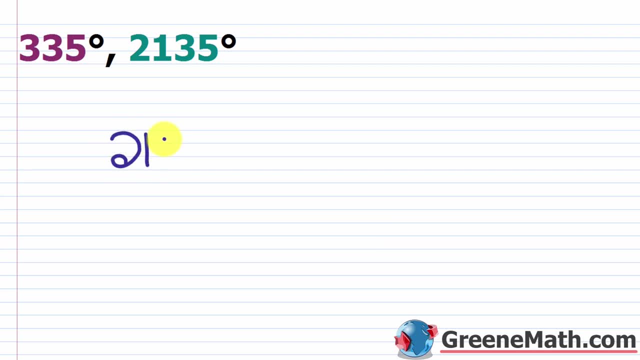 If I do 2,135,, 2,135 degrees minus 335 degrees, that's going to give me 1,800 degrees. Okay, Now, if I took 1,800 and divided by 360, I would get 5.. 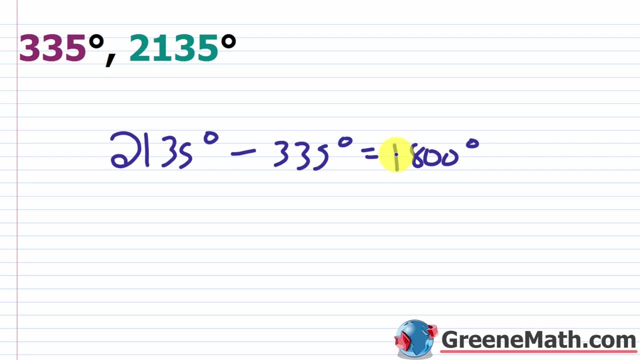 So we can say that their measures differ by some multiple of 360.. Okay, So they are going to be coterminal angles. Okay, Let's look at another example that you'll see in this section. So they'll tell you to find the coterminal angle. that is between 0 degrees and 360 degrees. 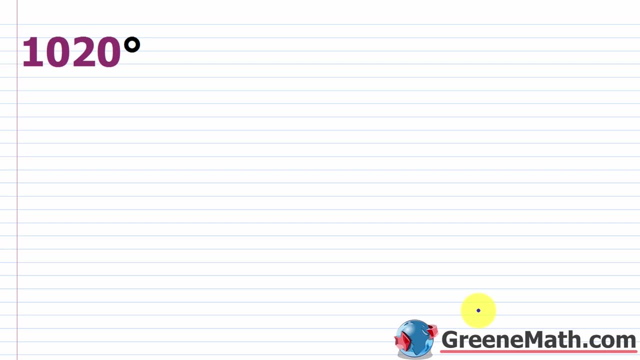 So for this guy there's kind of a slow way and a fast way. The slow way is to just keep subtracting or adding, depending on the situation. you're given 360 degrees until you get into the desired range. So I could subtract off 360 degrees and then do it again and I'd be in the desired range. 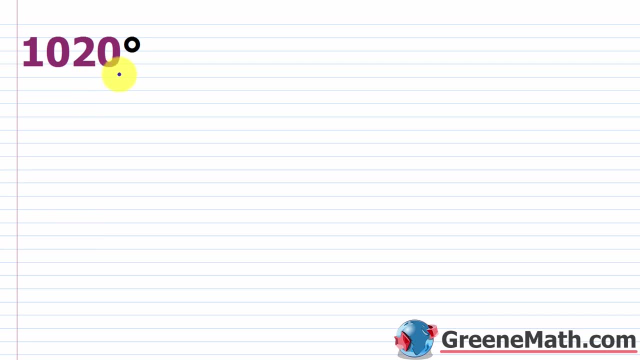 I can kind of eyeball that and say, okay, I'm going to subtract 360 degrees. I'm going to subtract 360 degrees, Okay. Well, if I subtract, it takes some nice round number. Let's say we take 400.. 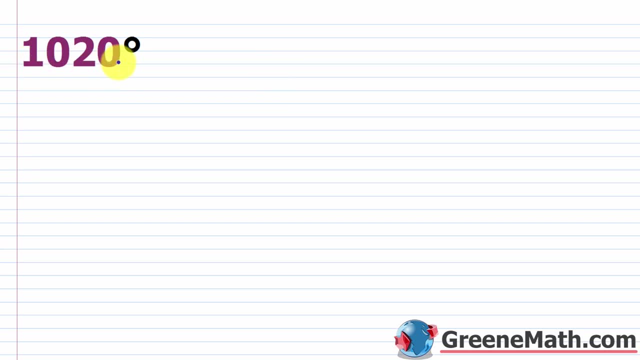 So I take 400 twice. Okay, That's 800. I know if I subtracted 1,020 minus 800, I'd have 220. So I'd know I'd be about where I need to be. So what I'm going to do is I'm going to take 360 and multiply it by two. 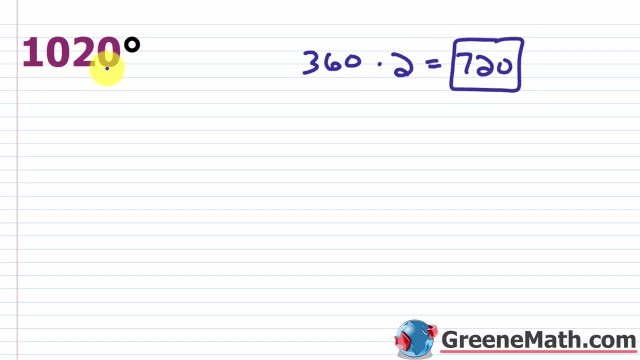 That gives me 720.. So this is the amount I want to subtract away from here Again. it's the same thing as if I subtracted away 360 and then subtracted away 360 again. Okay, That's all I'm doing. 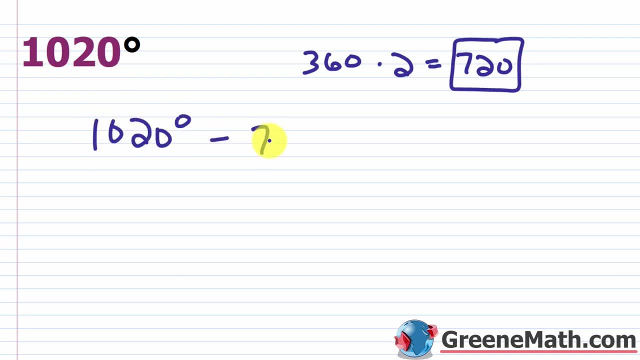 If I subtract away 1,020 degrees minus 720 degrees, this is going to give me exactly 300 degrees Okay, And we are in the range that we wanted between zero degrees and 360 degrees Okay. The last example is negative, 596 degrees. 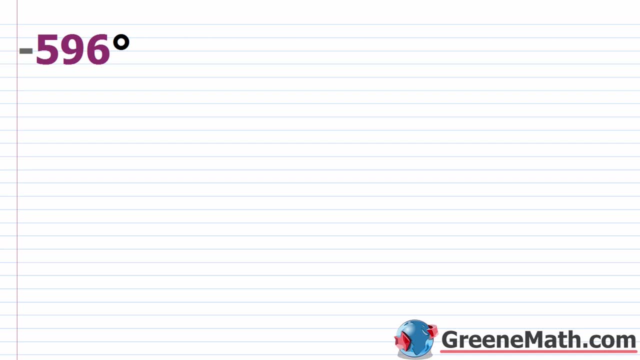 Again, if you want to find a coterminal angle where it's between zero degrees and 360 degrees- in this case you need to add- because it's a negative- 360 degrees until you get where you need to be. Okay. 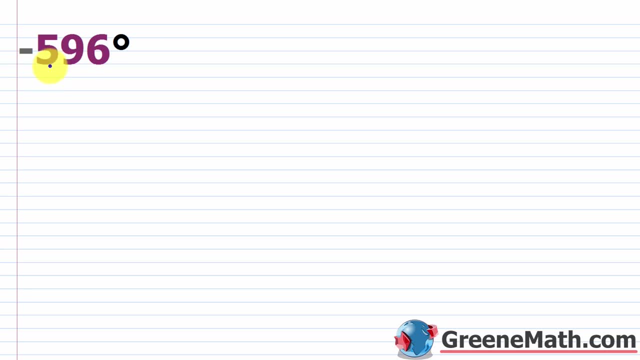 So if I add once, it's not going to be enough. Again I can just use 400 and say, okay, negative 596 plus 400, just approximating is going to give me negative 196.. So I know I'm not in the range with that, so I'd have to add again. 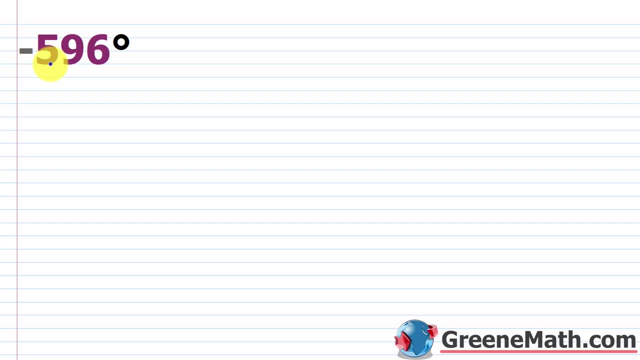 So if I add it again, I'd be at 204.. Okay, And that seems like that's where I want to go. Okay, So what I want to do is say: okay, I need two times 360, which again is 720.. 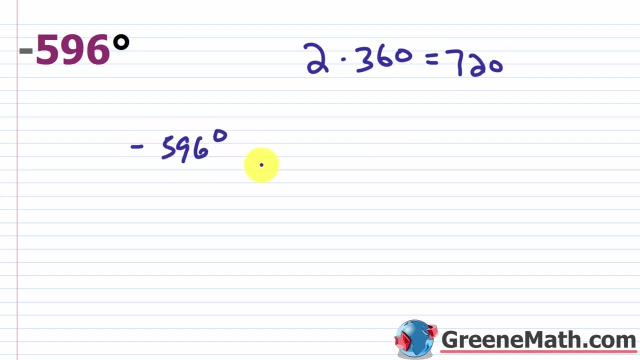 Okay, So I'm going to take negative 596 degrees and add 720 degrees. Okay, Of course, what you're going to do there is just subtract, right? So you would do 720 degrees minus 596 degrees, which would give me 124 degrees, right? 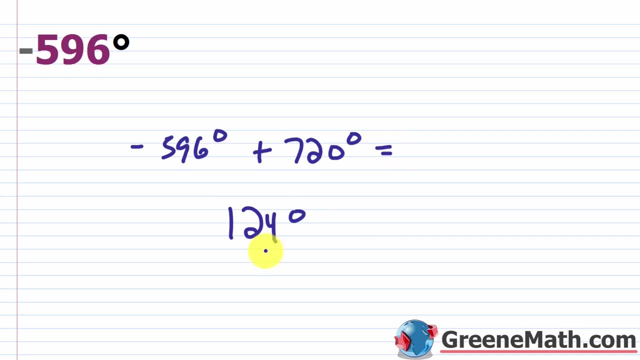 So in this case I'd have 124 degrees as my answer. This would be the coterminal angle with this guy. okay, that fits the criteria where it's greater than zero degrees and less than 360 degrees. In this lesson we want to talk about angle relationships and similar triangles. 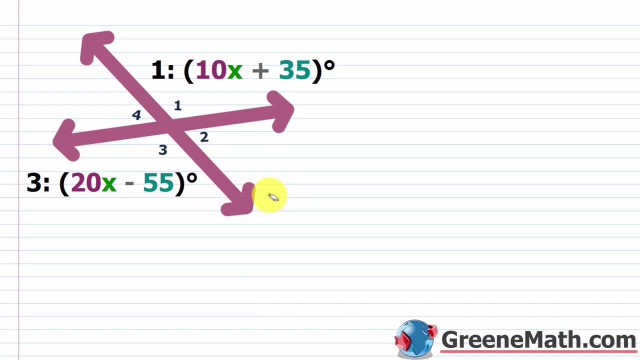 All right, For the first example, we're going to look at a problem that involves vertical angles. This is something very simple. Basically, vertical angles are angles opposite of each other, where the two lines cross. So you could see, here we have these two lines that cross and at this intersection point 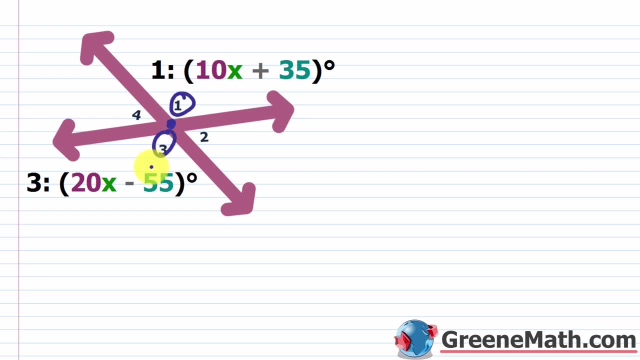 you have angles one and three that are across from each other. Okay, So those are vertical angles. And then you also have angles four and two that are across from each other. So those are vertical angles. right, You can show it like this, with matching arcs. 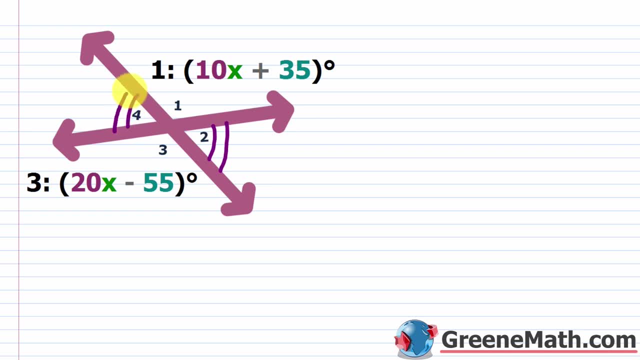 So I can just do two like this here And two like this here, And what I'll do is I'll do one here and one here, Okay, So angles one and three would have the same measure, and angles four and two will have the same measure. 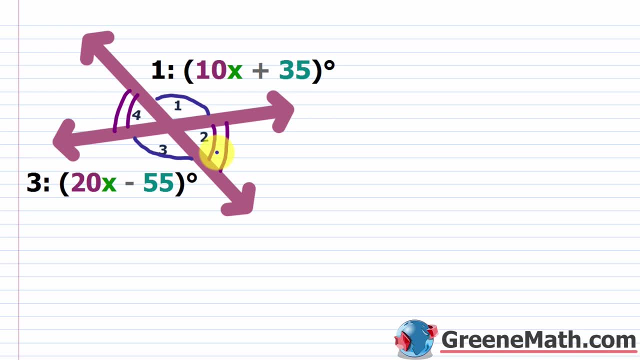 Okay, That's a property of vertical angles, Just saying that vertical angles are going to have equal measures. If we want to find the measure of angles one through four, what we do is we say, okay, we're given the measure of angle one, it's 10X plus 35 degrees. 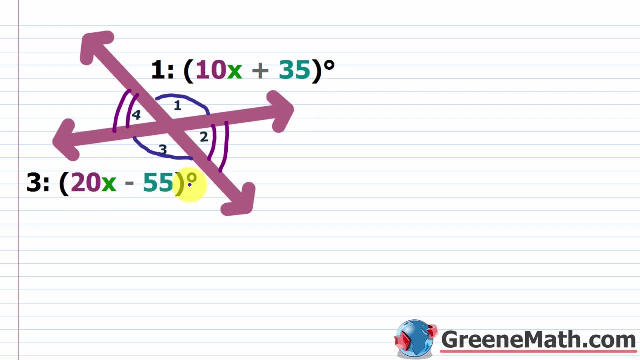 We're given the measure of angle three. it's 20X minus 55 degrees. Okay, What we can do is set angle one, which is again 10X plus 35 degrees, equal to angle three, which is 20X minus 55 degrees. 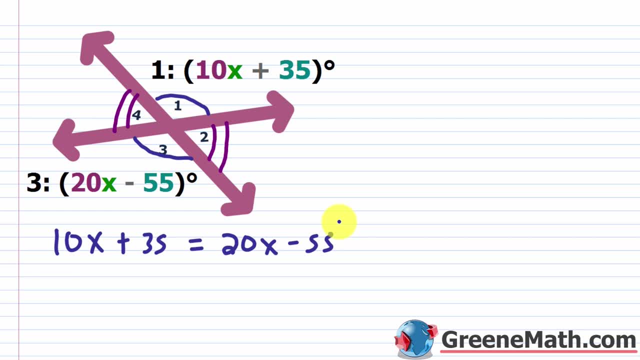 That's going to give me the value for X, And then I can plug that back in and find out what is angle one, what is angle three. So I'm going to go ahead and just subtract and let me scroll down and get some room. 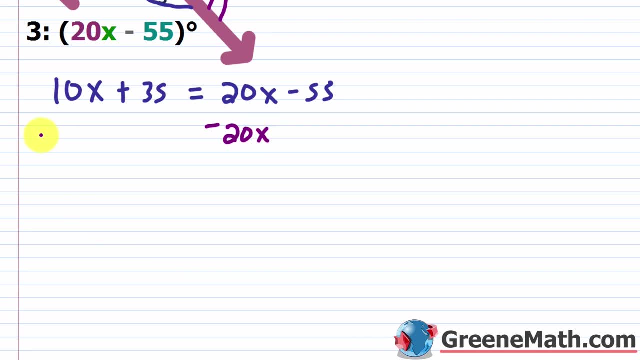 I'll come back up to the diagram in a minute. So I'm going to subtract 20X away from each side of the equation, And let's go ahead and get rid of this- And I'm going to subtract 35.. Okay, 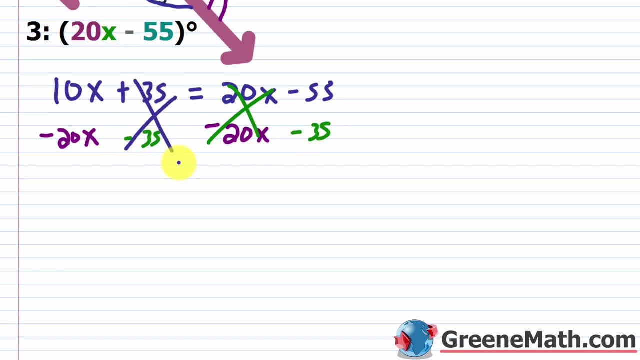 So I'm going to subtract 35 away from each side of the equation, So let's go ahead and get rid of this. And then if I do 10X- okay, 10X minus 20X, that's going to give me negative. 10X is equal. 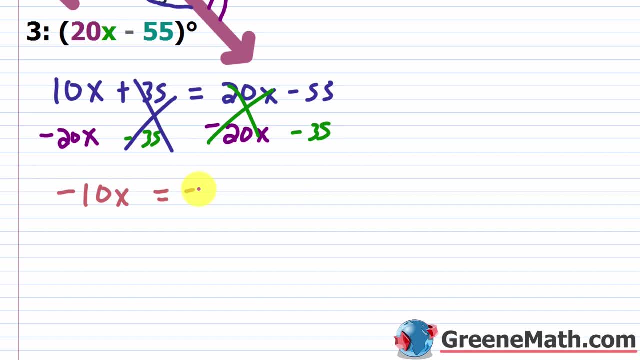 to negative. 55 minus 35 is going to be negative 90.. If we just divide both sides by negative 10, we're going to find that X is equal to not Okay. So let's erase everything, And if you're on a test or something like this, you just have to plug into one of these. 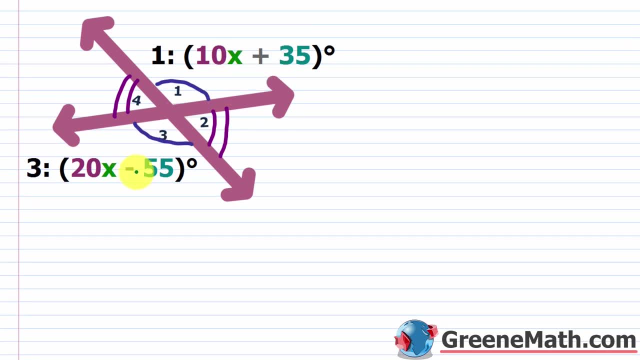 because, again, these are vertical angles, So the measure is the same. Okay, So we know that X is nine And if I plug in 10 times, nine is 90, 90 plus 35 is going to be 125.. Okay. 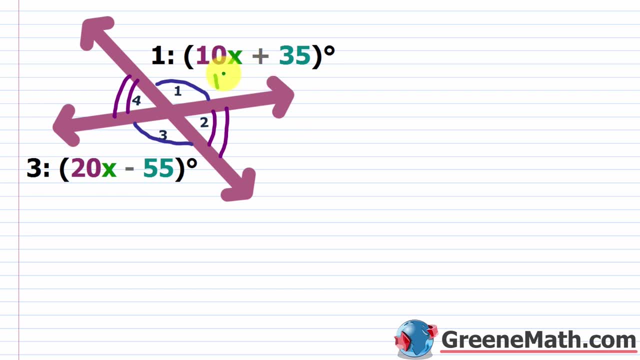 So the measure of angle one is 125 degrees- okay, 125 degrees. And also the measure of angle three is 125 degrees as well, Okay. And you could plug in there And again, if you plugged in a nine, 20 times nine is 180, 180 minus 55 is 125. 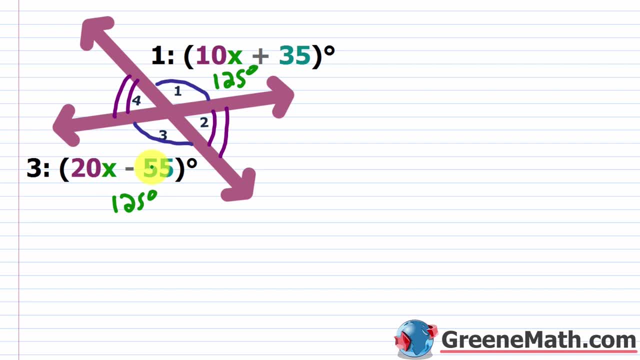 Okay, So that's where you get the 125 degrees. Now let's go ahead and get rid of this Now. the other thing that you would note here is that these guys, angles one and two, are going to be supplementary angles, right. 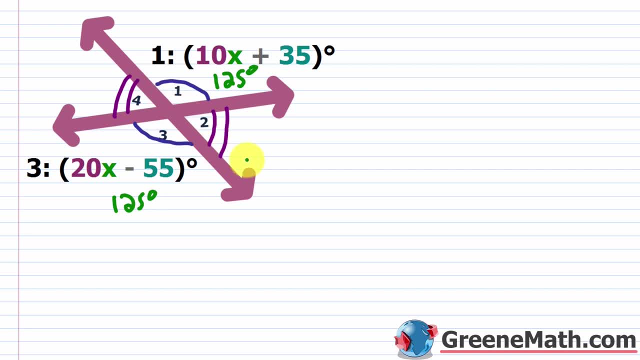 Their measure is going to add up to 180 degrees. If you kind of rotate this, you can see that this guy right here again, this is a straight line. Okay, This is a straight line. So if I took the measure of angles one and two, let me just do this as a full arc here. 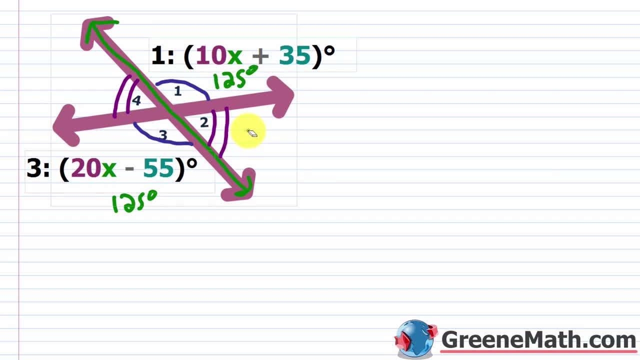 Okay, This would be 180 degrees. right, It would be a straight angle. Okay, So we know that the measure of angle two can be found. Okay, So we know that the measure of angle three can be found by taking 180 degrees and subtracting. 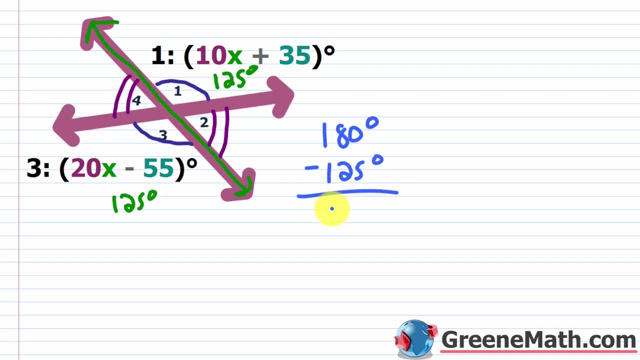 away 125 degrees, and that would give us 55 degrees. Okay. And again, because angles two and four are vertical angles, I can just put this as 55 degrees as well. Okay, So our answer for this problem is that we have 125 degrees for the measure of angles. 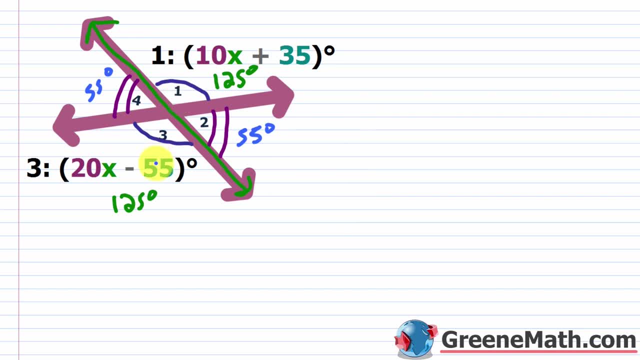 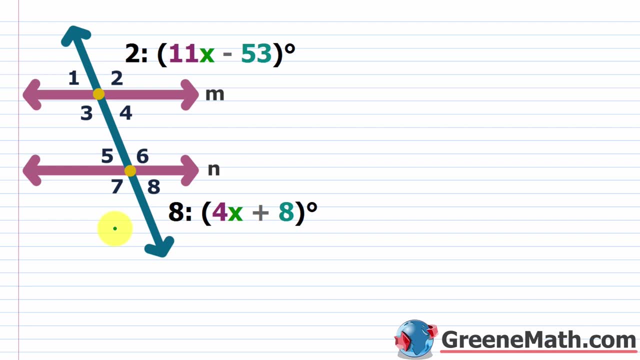 one and three, and then 55 degrees for the measure of angles two and four. All right, So let's look at an example that involves a transversal that intersects parallel lines. So we see that eight angles are formed here. You have one, two, three, four, five, six, seven, eight. 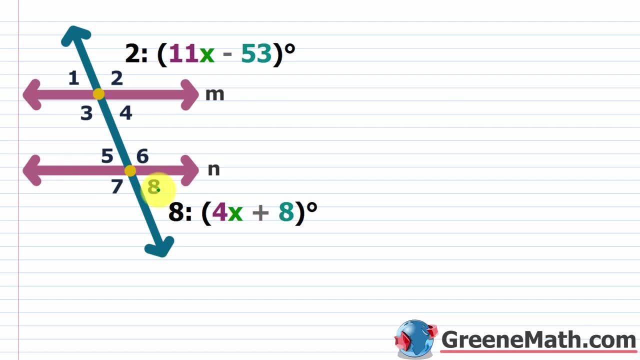 Okay, Those angles there have certain properties, So the ones I want to draw your attention to. we have interior angles, So you could think about this as being between the parallel lines, or some people say inside of the parallel lines. So those would be the angles three, four, five and six. 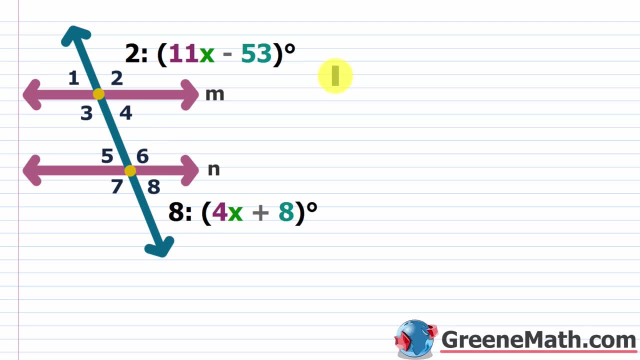 Okay, Okay, Okay. So those angles, they're going to have equal measure. Okay, So angles three and six, those would have equal measure. And then also- let me kind of change this up- also angles four and five would have equal. 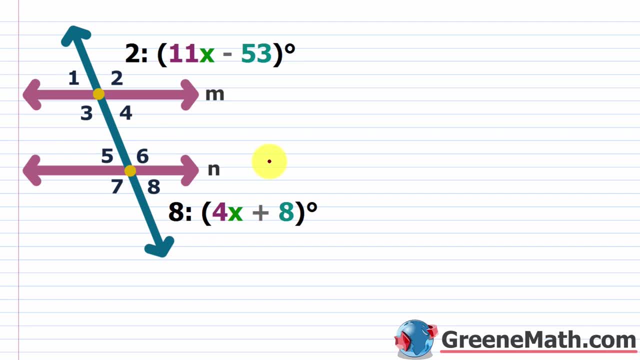 measures. Okay, So if we look at the alternate exterior angles, so the exterior angles would be- you can think about this as outside of the parallel lines, So angles one and two and then seven and eight- the alternate exterior angles will have equal measures. 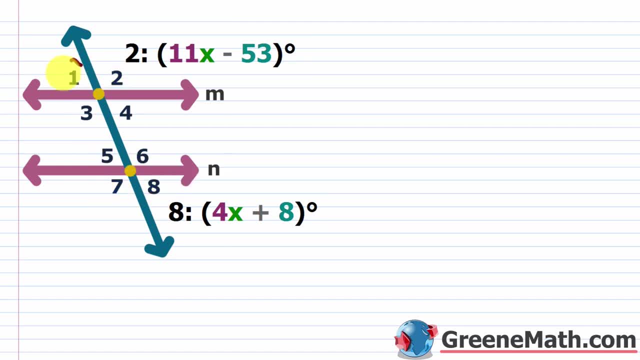 Okay, So we can say that would be angles one and eight. Okay, And then also we can say angles two and seven: Okay, So we can use these properties to find out the value for all eight angles here. So if we start out with the fact that angle two has this measure, 11X minus 53 degrees. 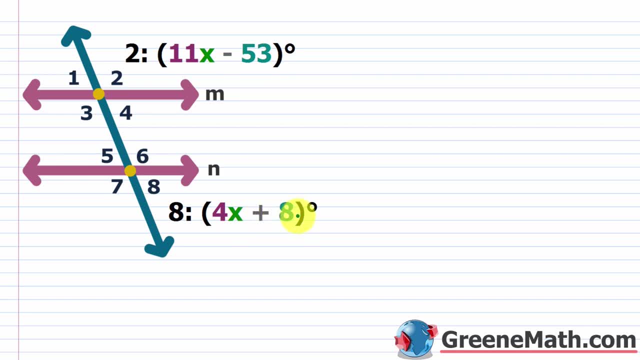 and angle eight, has this measure four X plus eight degrees. Well, let's think about the fact that angles two and seven are alternate exterior angles, right Alternate exterior angles, So they would have the same measure. Okay, So we can write that the measure of angle seven is 11X minus 53.. 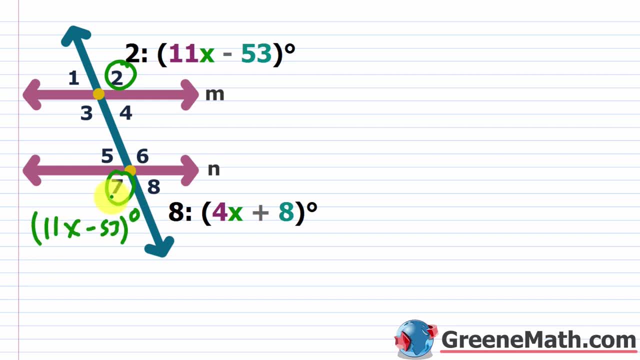 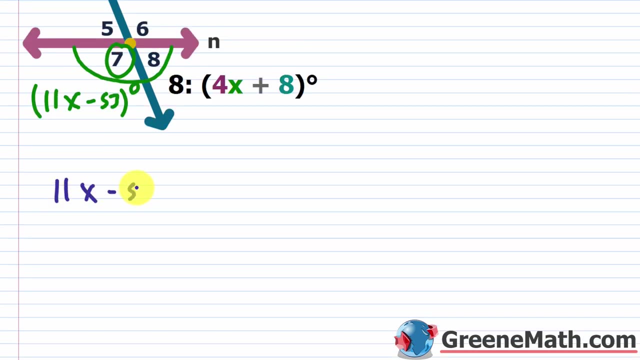 Okay, Degrees. Okay. So we know that angles seven and eight together form a straight angle right, Or an angle that's 180 degrees. So in other words, angle seven and eight are supplementary angles. So what I can do here, I can add 11X minus 53 plus four, X plus eight and set this equal. 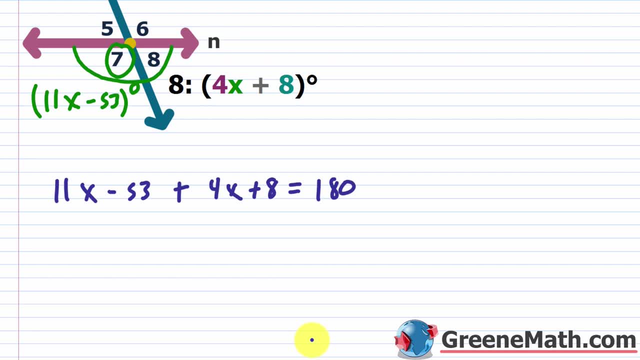 to 180.. Again, for 180 degrees, I can solve for X. I can go back and plug in and find out what is the measurement of each angle, one through eight. Okay, So what I'm going to do here, 11X plus four X is going to be 15X, and then negative 53. 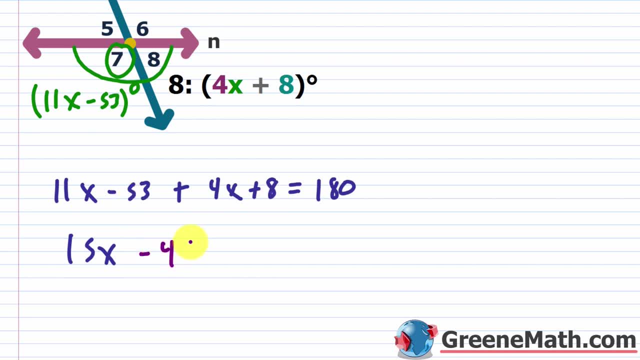 plus eight is going to give me negative 45. So minus 45, this equals 180.. Okay, So if I add 45 to each side of the equation, let me scroll down and get some room going- Then what am I going to have? 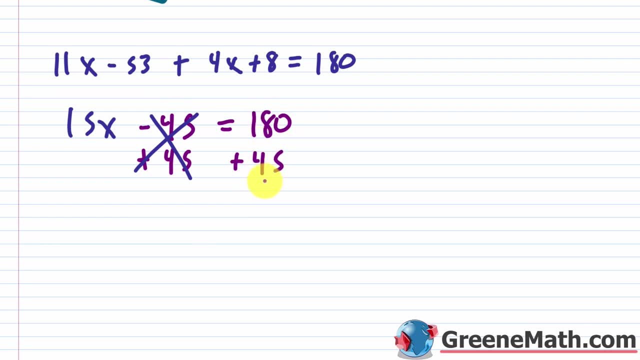 This is going to cancel. And if I do 180 plus 45. Okay, I'm going to get 225, and this over here is still 15X. If I divide both sides by 15, I'm going to get that X is equal to 15.. 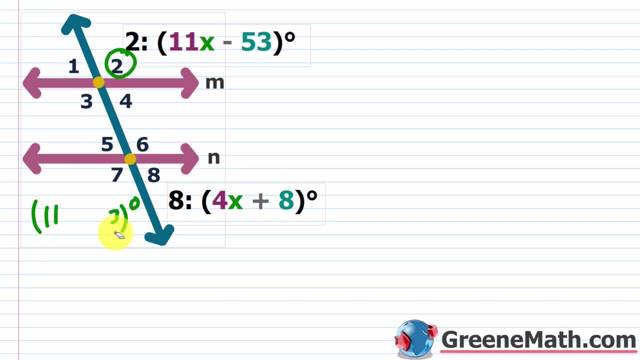 Okay, So let's erase this and we're just going to plug in. We can get rid of this. Okay, We're going to plug in a 15, starting here. So what is 11 times 15? That's going to be 165.. 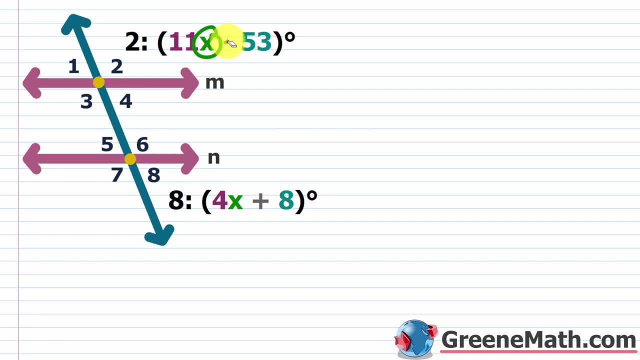 And if I subtract away 53, I get 112. So I know that the measure of this guy is 112 degrees. Again, alternate exterior angles: Okay, Okay, Alternate exterior angles have the same measure. Okay, So this guy. two and seven have the same measure. 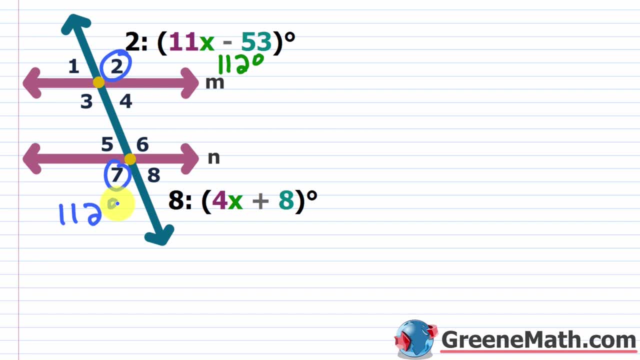 This is 112 degrees. here, Remember that vertical angles have the same measure, So that means that seven and six have the same measure. Okay, So this is 112 degrees. Two and three have the same measure, So this is 112 degrees. 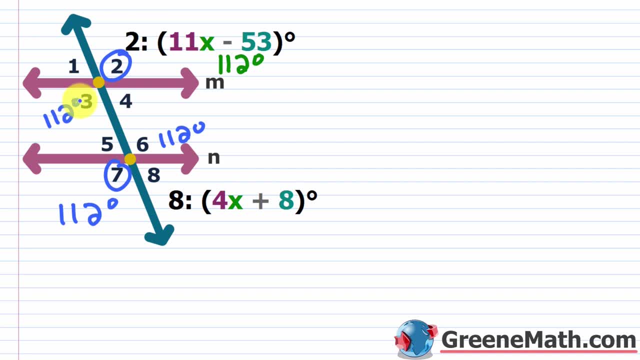 Okay, So at this point you know four of your angles and again you can figure out the rest. You can plug in here If you want. you can plug the 15 in and do it that way, Or you can just take 180 and subtract away 112 and get 68 and fill out the rest, right. 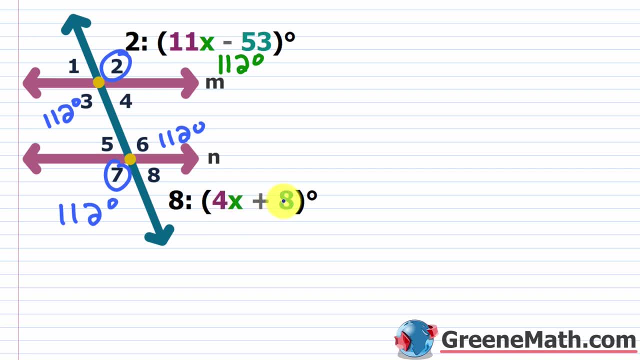 Because again, if I plugged in a 15 there four times 15 is 60,, 60 plus eight is 68. So this is 68 degrees. Or again you can use the fact that seven and eight are supplementary angles. 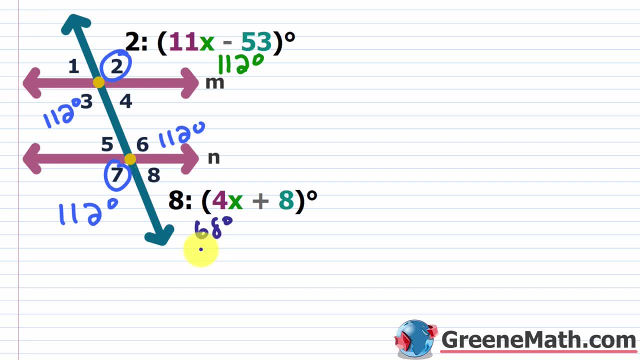 So you can subtract 180 minus 112 to get the 68 as well. Now again, eight and one are alternate exterior angles, So they have the same measure. And then again you can also say that one and four are vertical angles. 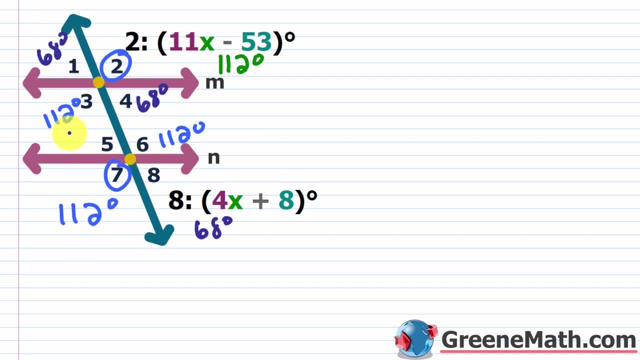 So they have the same measure. And eight and five are vertical angles, So they have the same measure. Okay, And there's lots of different ways to go about getting these values, but you can see that for angles one, four, five and eight, the measure of the angle is 68 degrees. 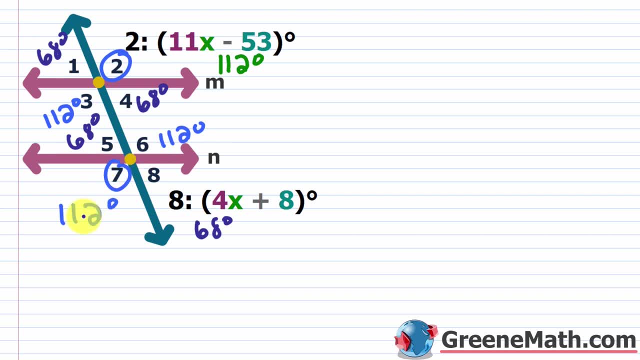 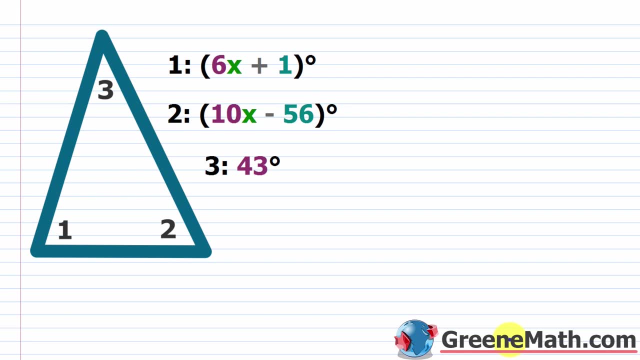 And then for angles two, three, six and seven, the measure is going to be 112 degrees. All right, So let's look at some examples now that involve triangles. So what you need to know here is that The sum of the measures of the angles for any triangle is going to be 180 degrees. 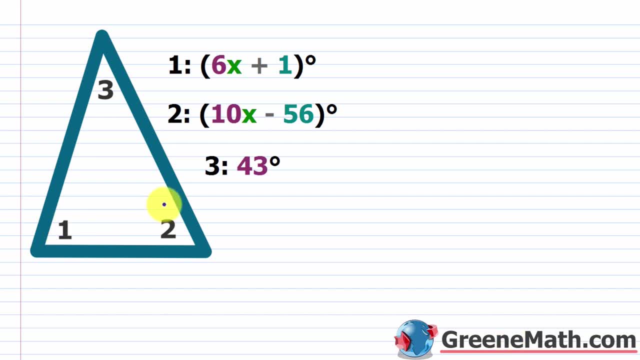 So with this example, here we're given angles one, two and three, and the measure of angle one is six X plus one degrees. The measure of angle two is 10 X minus 56 degrees And the measure of angle three is given it's 43 degrees. 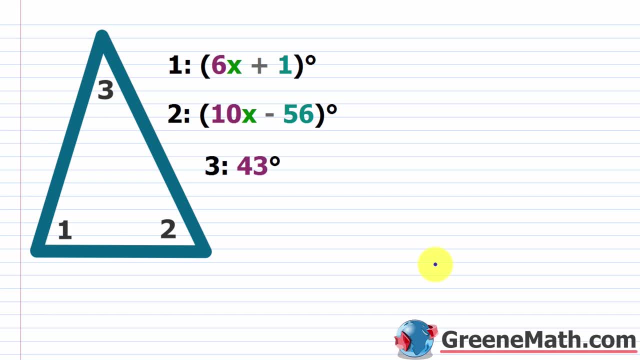 So all we really need to do is set these guys as a sum, and it will be equal to 180 degrees. Okay, So if we set up a sum here, So we'd say six X plus one Plus 10 X minus 56.. 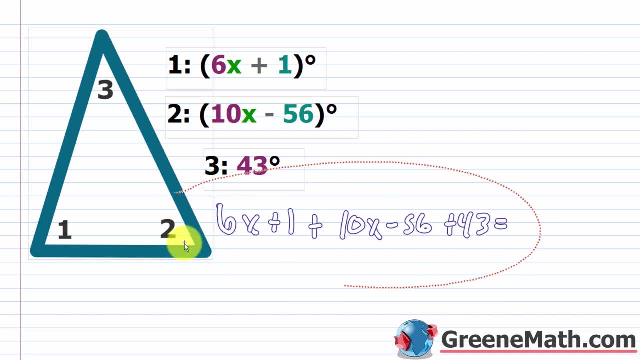 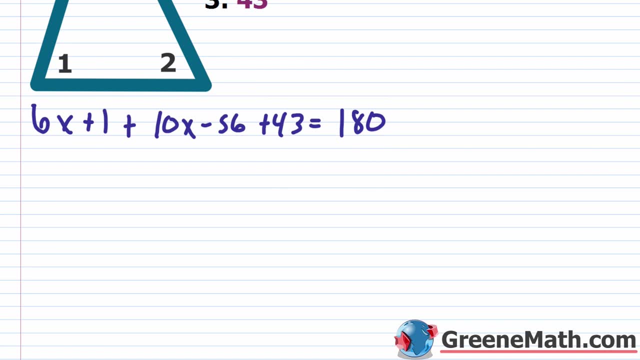 Then plus 43. And this will be equal to- let me drag this down, cause I'm going to run out of room here And let me just get some room going- So this will be equal to 180.. Okay, And we just solve for X. 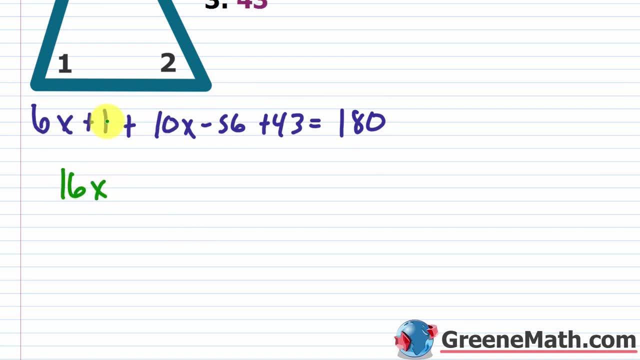 Very simple. So six X plus 10 X is 16 X. One minus 56 is going to be negative 55. Then negative 55 plus 43 is going to be negative 12. So I'll put minus 12 here. 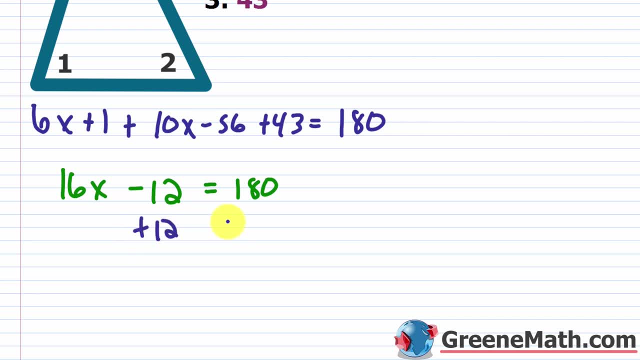 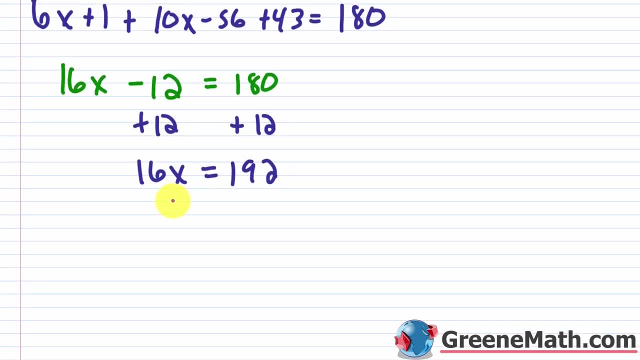 This equals 180.. If we add 12 to both sides of the equation, we're going to get that 16 X is equal to 192, and get some room going here. To finish things off, I'm going to divide both sides by 16 and get that X is equal to. 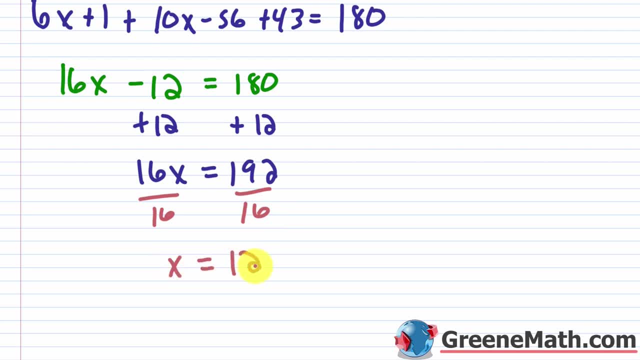 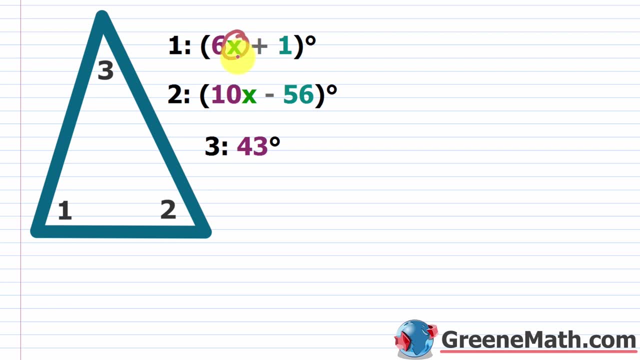 12. So X is 12 here. So let me erase all this. So we said that X was 12.. So for angle one, if I plug in a 12 there six times 12 is 72,, 72 plus one is 73.. 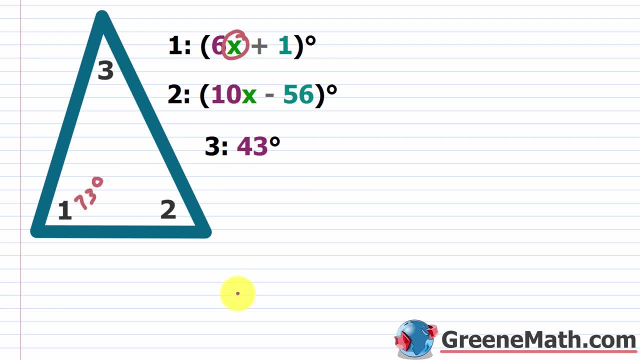 So the measure of angle one is 73 degrees. Okay, So I'm going to put it here as well: This is 73 degrees. For the measure of angle two, it's going to be 10 times 12, which is 120 minus 56,, which. 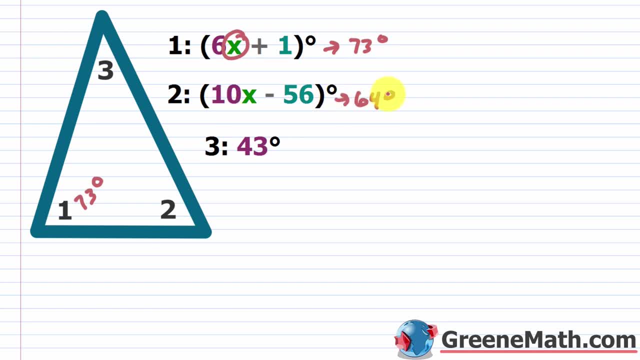 is going to be 64.. Okay, So this will be 64 degrees And I'll write that in here. This is 64 degrees. We're already given the fact that this is 43 degrees And again, if you sum these amounts, you're going to get 180 degrees. 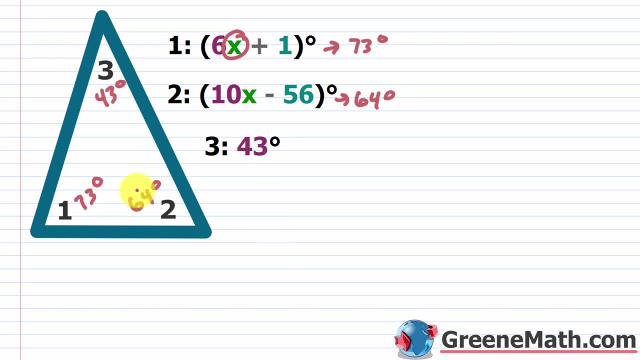 All right. For the next two problems, we're going to see typical examples where we're dealing with similar triangles. So hopefully you remember this from geometry. but essentially, if you have a triangle, you're going to have a triangle, You're going to have a triangle. 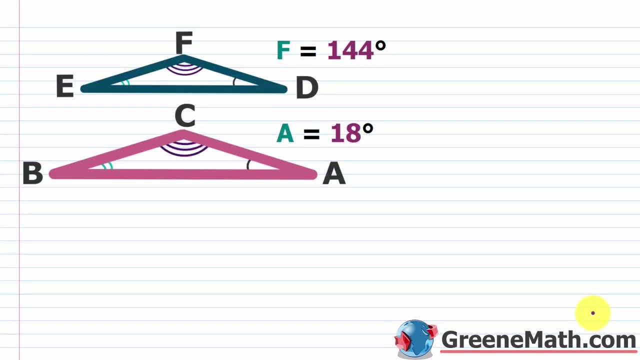 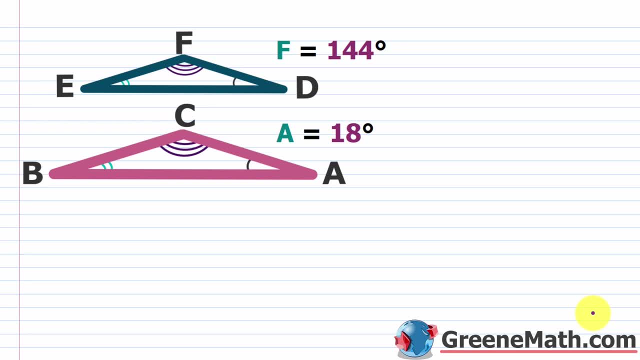 then corresponding angles must have the same measure. Okay, Then, secondly, corresponding sides must be proportional, So that means the ratios of their corresponding sides must be equal. Okay, So for the first problem, we're going to deal with a statement that says that corresponding 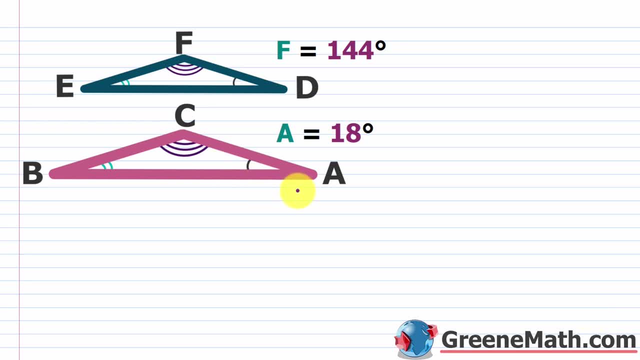 angles must have the same measure. Okay, So we have these two similar triangles. So this is extremely difficult and I'm just going to call this first one triangle ABC. So I'll say triangle ABC is similar to triangle DEF. Now what you want to do is match up the corresponding angles. for this problem. 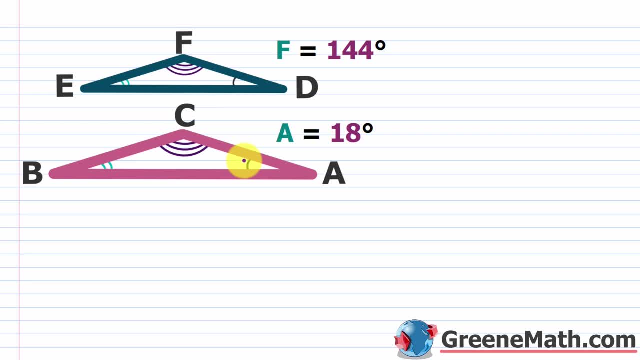 You'll notice that the corresponding angles have matching arcs. Okay, so we have one arc here and one arc here. So angle A corresponds to angle D, and then you have two arcs here and two arcs here. So angle B corresponds to angle E, and then you have three arcs here and three arcs here. So 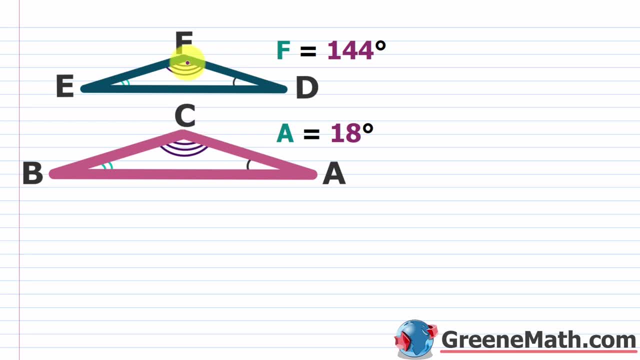 angle C corresponds to angle F. Now, as we just said, corresponding angles. if you have similar triangles, they must have the same measure. So what that tells me is that if I know the measure of angle F is 144 degrees, then I also know the measure of angle C is going to be 144 degrees. 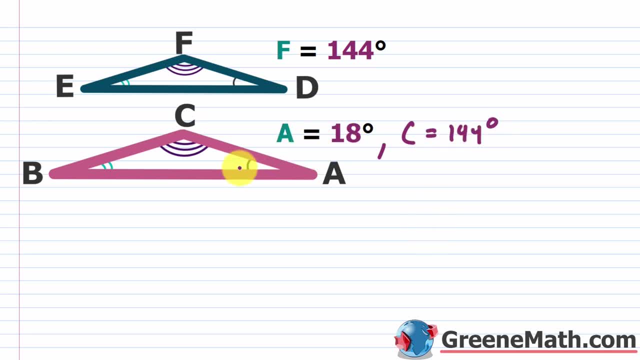 as well. If I know that the measure of angle A is 18 degrees, that tells me that the measure of angle D is 18 degrees as well. Now, what I don't know here is the measure of angle B and the measure of angle E. So let me fill out this guy right here. I'll just put E and I'll put. 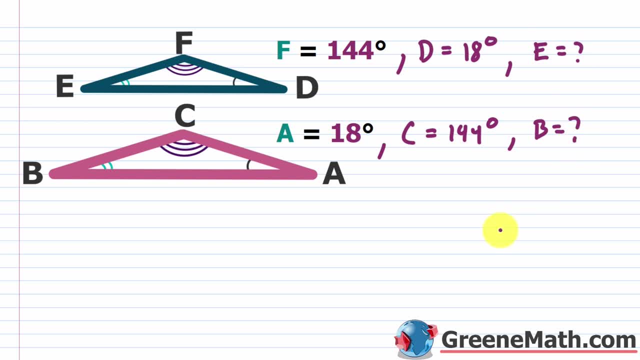 a question mark, and for this one I'll put B and put a question mark. Now, how can we figure this out? Remember, when we think about the sum of the measures of the angles of any triangle, it's going to be 180 degrees. So what I could do is take 180 degrees and subtract away the sum. So, in each case, 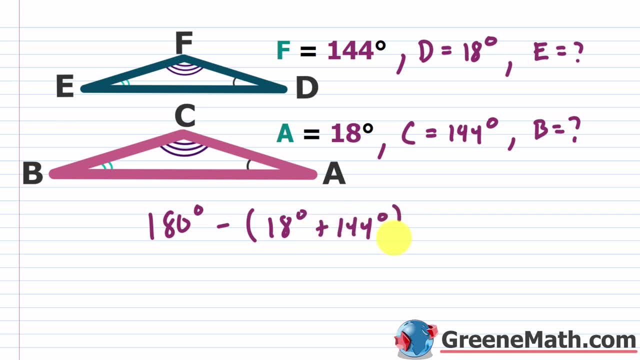 it's 18 degrees plus 144 degrees, So this sum represents the angle measures. for two angles, 180 degrees would be the sum of all three. So if I take this one, subtract away the sum of the two, I'm going to get the missing one. So let's put this as equal to: so 18 degrees plus 144 degrees. 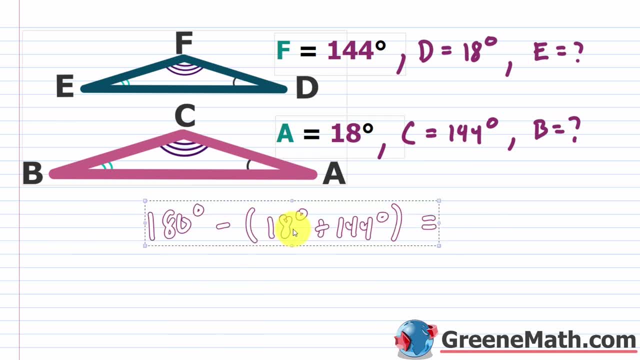 that would be 162 degrees. So this- let me just slide this down- would be 180 degrees minus 162 degrees, which gives me 18 degrees. So if we're trying to find the measure of angle B, it would be 18 degrees. and again, because angle B corresponds to angle E, they're going to have the same measure. 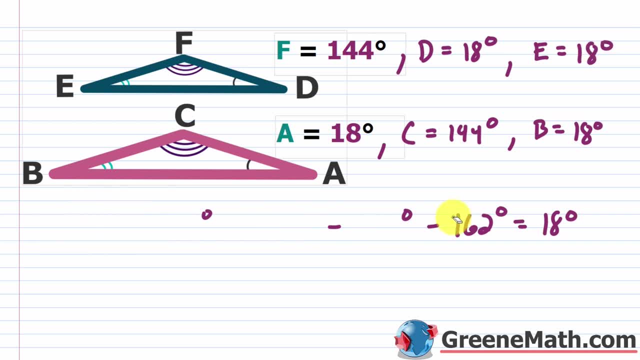 so this is 18 degrees as well. So, if you wanted to know the angle measure for all of these guys, well, in this bottom triangle, the measure of angle A is 18 degrees, the measure of angle B is 18 degrees as well, and the measure of angle C is 144 degrees. and then, in the top triangle, the 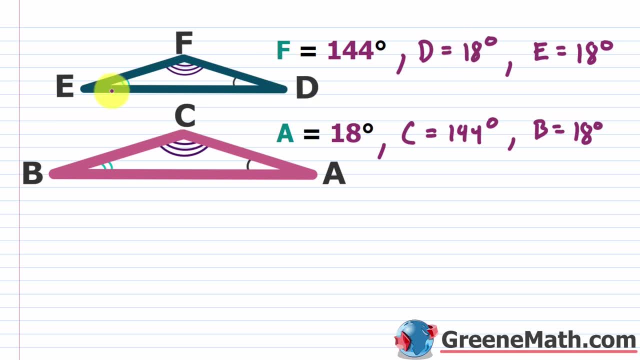 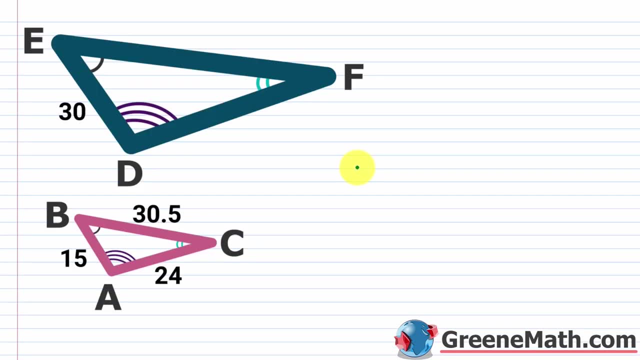 measure of angle D is 18 degrees, the measure of angle E is 18 degrees and the measure of angle F is 144 degrees. All right for the last problem. here let's look at an example with similar triangles where we're asked to find some missing side lengths. So this is a very easy problem to solve. 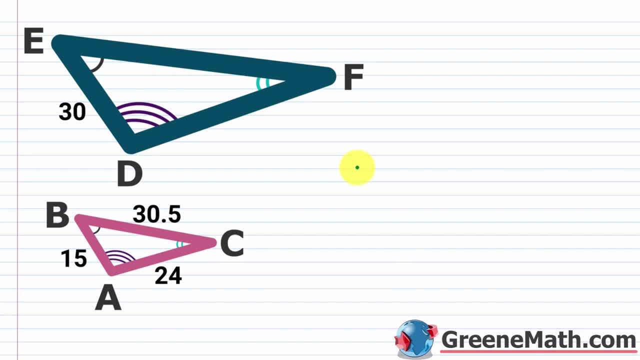 just deals with proportions and essentially what you're going to do here is look at these two guys and generally you're going to be given a statement that says something like: triangle ABC is similar to triangle DEF. Now we already know about finding the corresponding angles. You could do it based on. 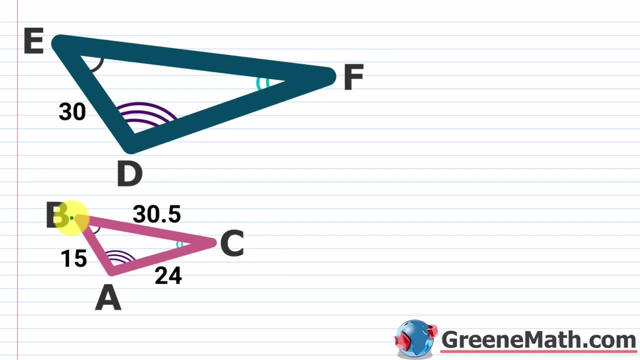 the way that I read the two triangles. So again I said triangle ABC is similar to triangle DEF. so that tells me that triangle DEF is similar to triangle DEF. So that tells me that triangle ABC is similar to triangle DEF, that A is going to correspond to D, B is going to correspond to E and C is going to correspond to F. 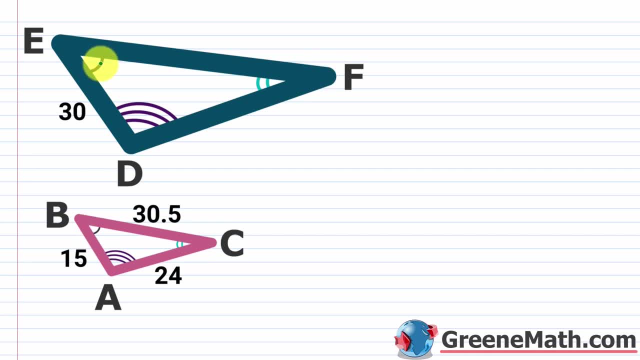 Or again, you can use those matching arcs. So you have a single arc here and a single arc here, So B and E are going to correspond. You have a triple arc here and a triple arc here, So A and D are going to correspond, And then a double arc here and a double arc here, So C and F are going to. 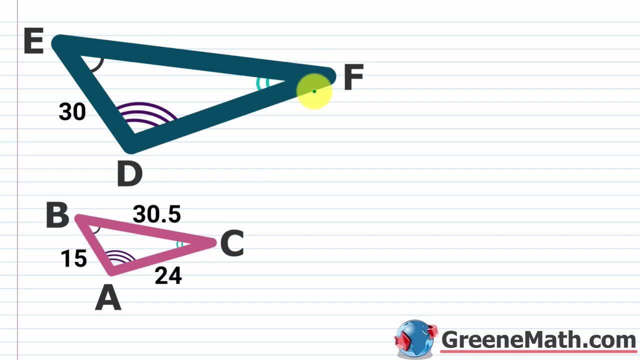 correspond. Now, when it comes to side lengths, a lot of times you just have to write things down. if you're given a not so easy scenario Here, it's very easy, you can match things up, but sometimes triangles are flipped all the way around and stuff like that, so it's not so easy. So you might want to. 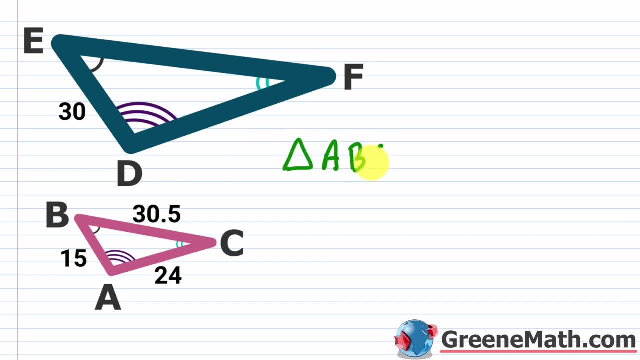 write the statement out and say: triangle ABC is similar to triangle, in this case DEF, And then you can just match things up So I can say this side AB is going to correspond to this side DE. So here's my side AB, Here's my side DE. Those are corresponding sides. Then I have the side BC. 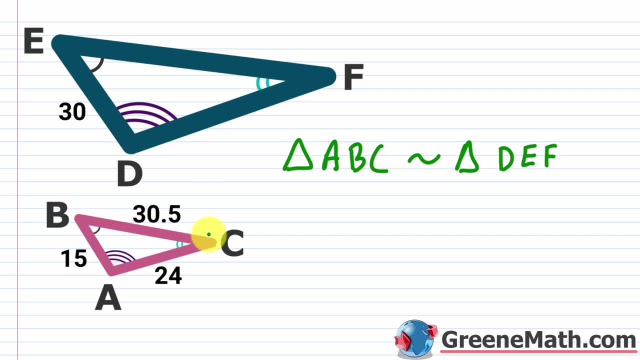 that's going to correspond to the side EF. So here's my side BC, my side EF. you can see those are corresponding sides. And then, lastly, you can say this side AC is going to correspond to the side DF. So here's my side AC, my side DF. those are corresponding. 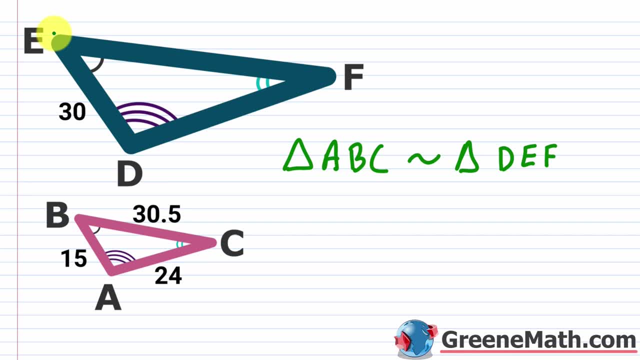 sides. Now we know, if we're working with similar triangles, that corresponding angles must be equal and corresponding sides must be proportional. So again, this just means that the ratios of their corresponding sides must be equal. So let's use that to set up a little proportion. 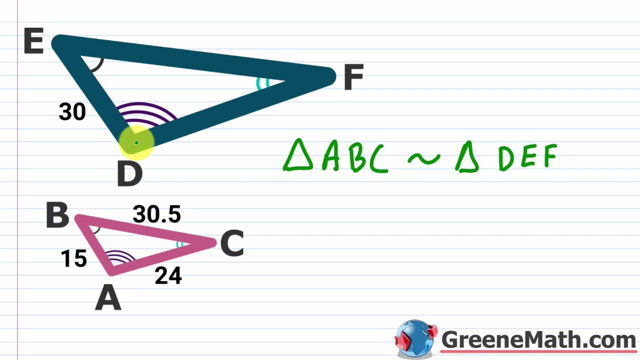 So I know that this side AB corresponds to this side DE. Okay, so what I'm going to do is write the ratio of the length of this side AB to the length of this side DE. So I'm going to set that up as a fraction. I'll just say: this is AB, So that's going to denote the length of this side. 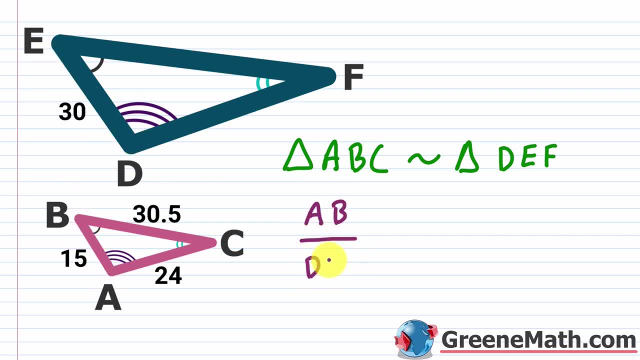 to this will be DE, So that'll be the length of this side. I'm going to say that's equal to the ratio of. let's go ahead and say the length of the side BC. So the length of the side BC, the length of the side BC, to the length of the side EF, So the length of the side EF. So let me. 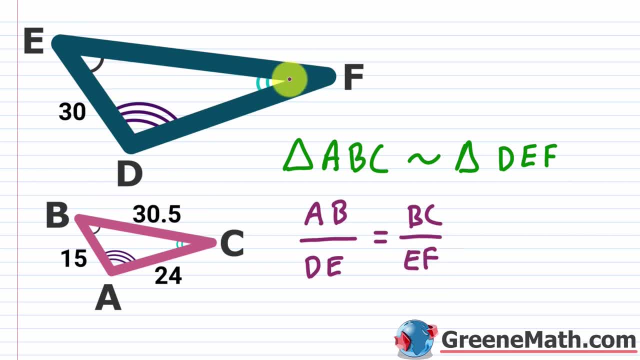 write that in there. And again, we know that BC and EF are corresponding sides And I'll also say: this is equal to the ratio of the length of the side AC, So that's going to be right here. So AC to the length of the side DF, So DF is going to be right there. So once you have this set up, 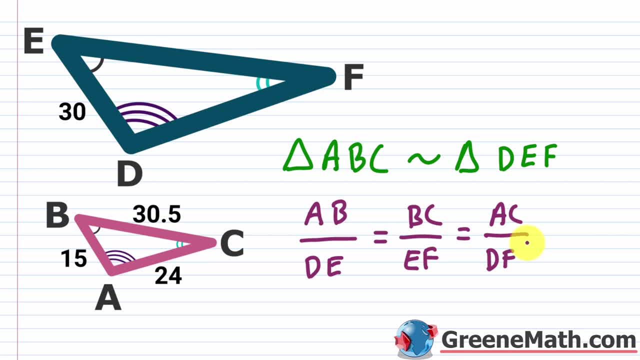 I would go through and plug in what you can And then you're just going to solve the equation. So I'm going to go through and plug in what you can And then you're just going to solve for what you don't have. Okay, Now, before I even do that, a lot of people are 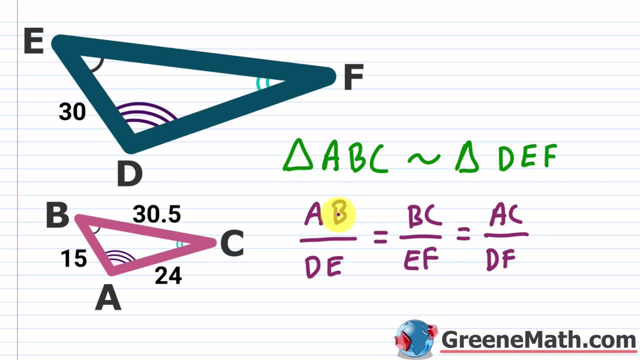 going to ask: why did I choose to put the AB on top and the DE on the bottom here? And it actually doesn't matter. you could flip this, but you have to stay consistent. In this case, I wrote the information from the smaller triangle over the information from the bigger triangle, But I could 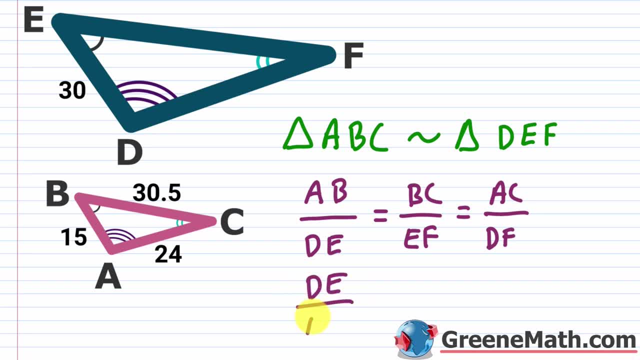 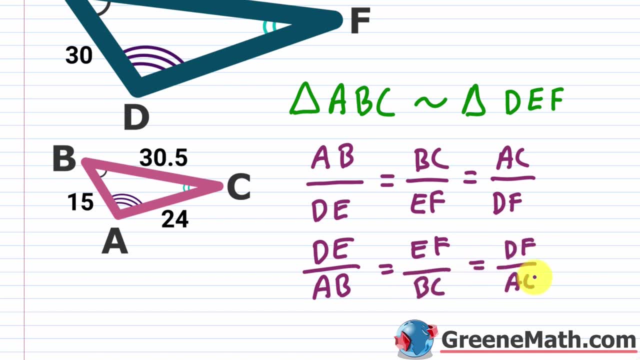 have also set this up as DE over AB is equal to EF over BC, is equal to DF over AC. Okay, so, as long as you stay consistent, you're going to be able to solve the equation. So let's go ahead and consistent, you're going to be good to go. So I'm just going to keep it like this And I'm just 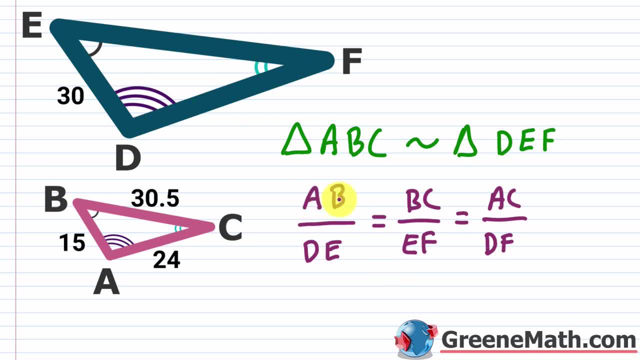 going to replace what I can. So for the length of this side AB, it's 15.. So I'm just going to replace this with 15.. For the length of the side DE, it's 30. So I'm going to replace that with 30.. 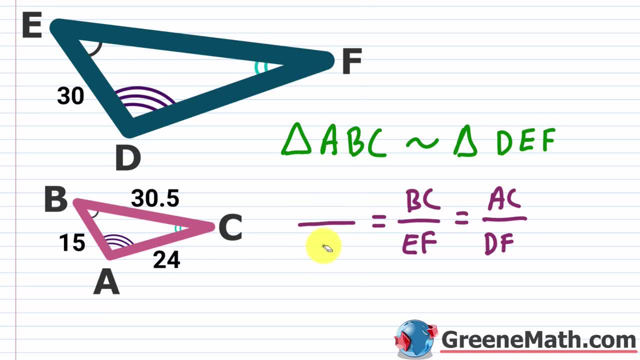 Now, 15 over 30 is one half. So let's just simplify that and say it's a half. Now for the length of the side BC, it's 30.5.. So let me put that in. And then for the length of the side EF, that's an unknown right, So we don't know the length of. 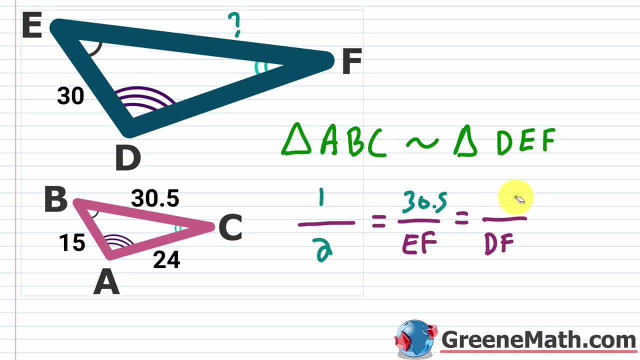 that side. And then for the length of the side AC, that's 24.. So this is 24.. And for the length of the side DF, that is unknown. Let's grab this real quick And I'm just going to solve one of these at a time. 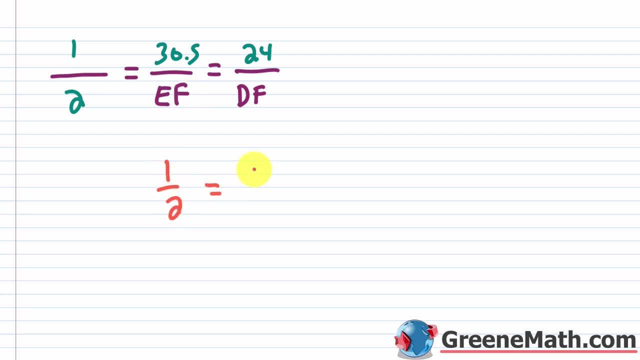 So I'm going to pick the one on the left and say one half is equal to 30.5.. This is over Again. the EF is the length of the side EF. So cross, multiply and you will get EF is equal to two. 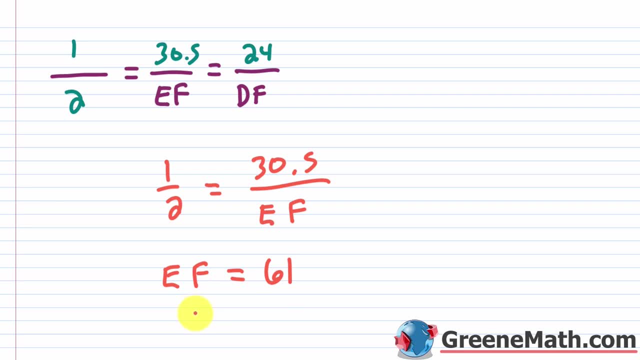 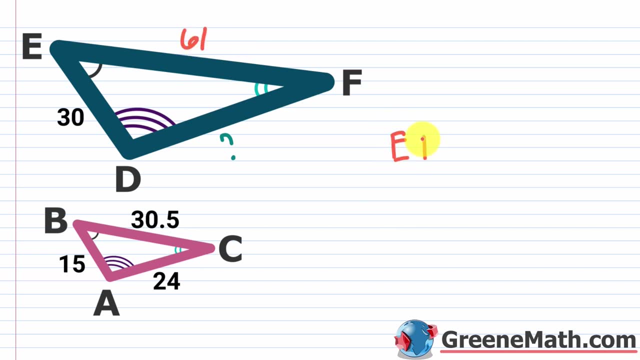 times 30.5 is 61. So the length of the side EF is 61. So you can come back up here and just put that this is 61, right here. Or, if you wanted to notate this, you could say EF. this just stands for the length of. 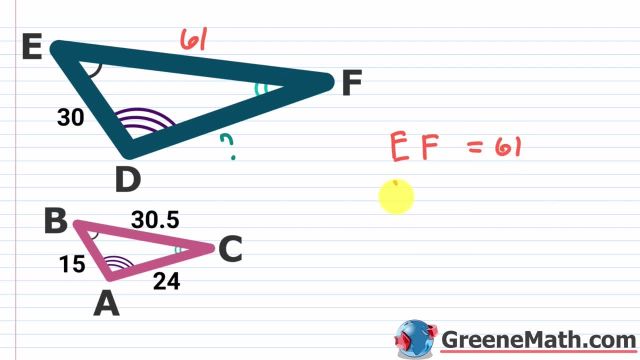 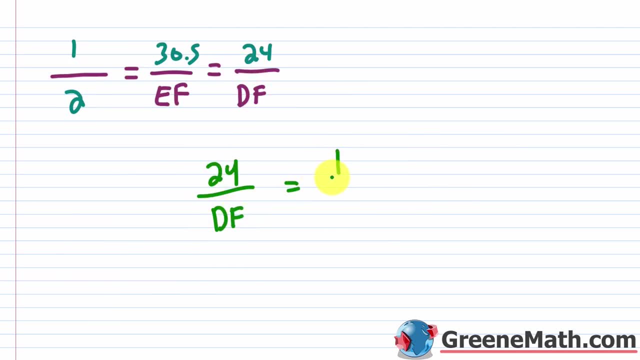 the side EF, that's going to be 61. Okay, let me put DF here And we'll come back down. So I'm going to set 24 over DF, equal to a half. you wouldn't want to set this equal here because you're not. 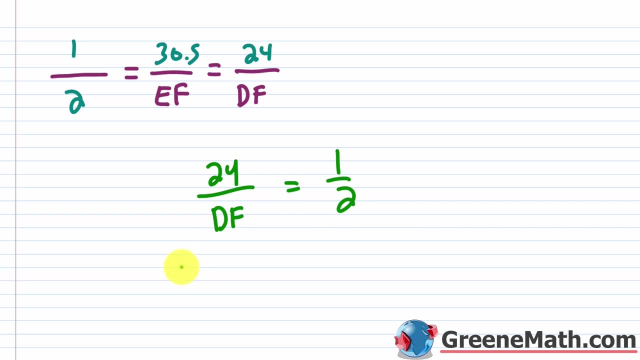 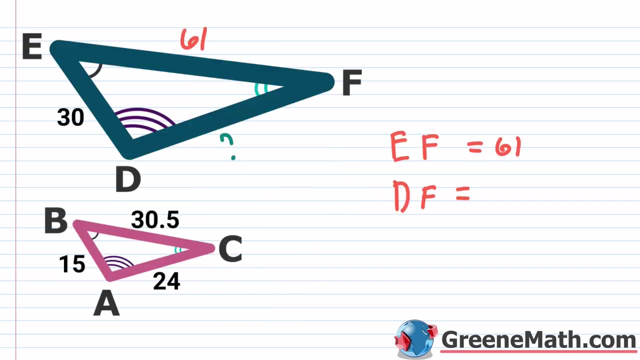 going to be able to solve. So I'm going to cross multiply again. So this is: DF is equal to two times 24 is 48. So the length of that side, DF, is going to be 48. So coming back up, you can put 48 here. 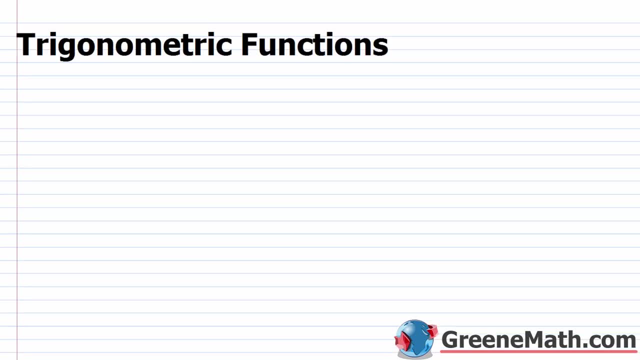 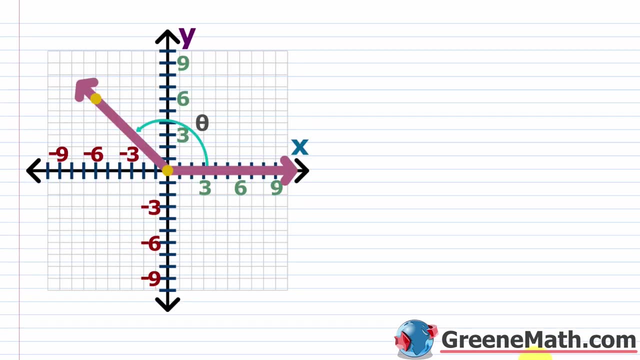 and 48 here In this lesson we want to talk about the trigonometric functions. All right, so to define our six trigonometric functions, we're going to start with an angle in standard position And we're going to name this guy using the Greek letter, theta. So you have your angle. 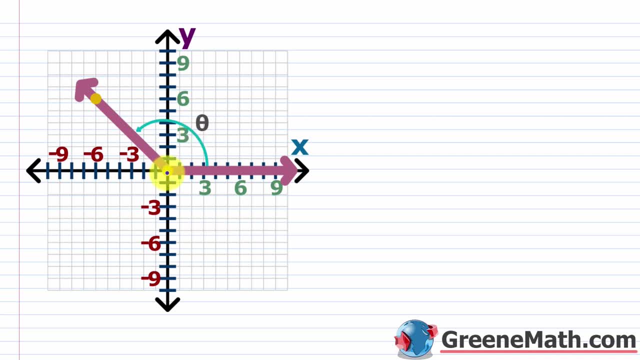 theta there. Remember, in standard position your vertex is at the origin, your initial side lies on the positive axis and your vertex is at the negative axis. So you're going to start with an X axis. So this is your initial side, And then this guy over here is called your terminal side. 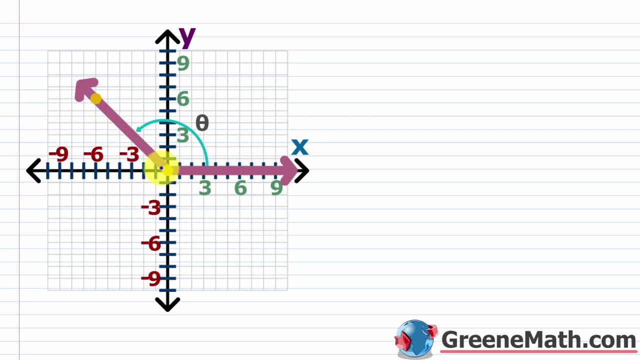 So what we're going to do from here is we're just going to pick some point. okay, that's not the origin, that lies on the terminal side. So this point that I've chosen here could be any, but I've chosen this one. this is going to be the point which is negative. six comma six, so negative. 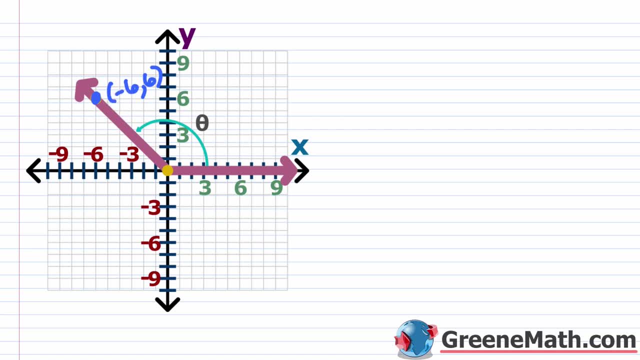 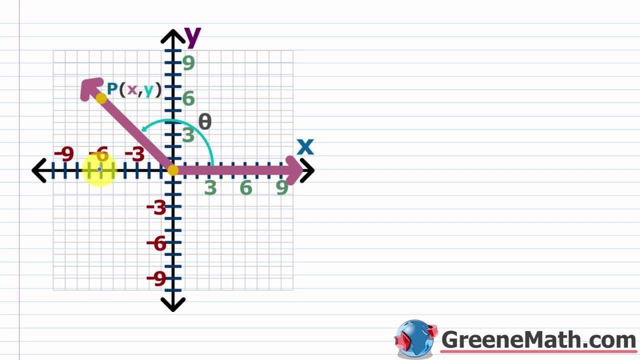 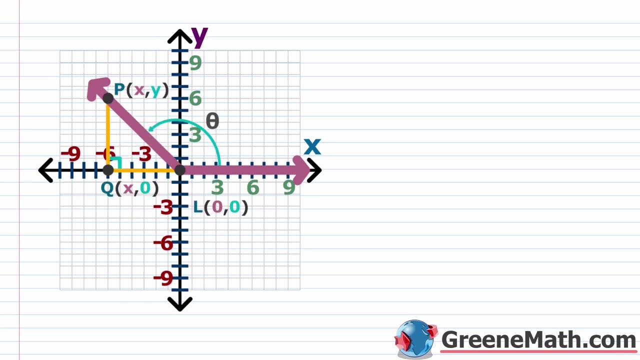 six comma six. Now for the formulas. you want something generic, So what I've done is I've just labeled this as point P with the coordinates x comma y. of course, you can fill that in with whatever you have. Here we have negative six for x and positive six for y. Now, additionally, what we need to do to get: 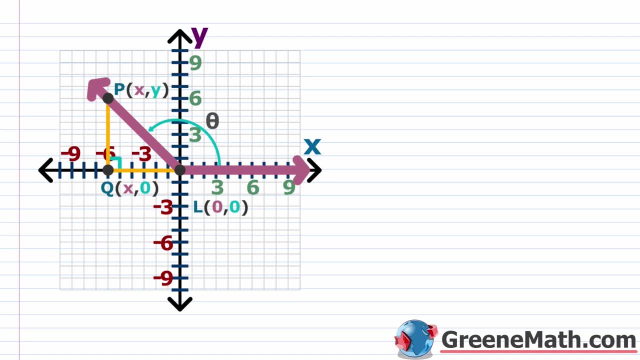 started is we need to know about something called r. okay, So r is just going to take the place of d in the distance formula. So you remember that the distance formula, the distance between two points in the coordinate plane, is equal to the square root of you have your x sub two minus x sub one. 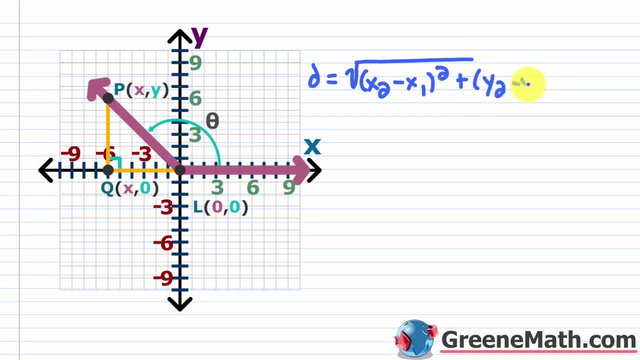 quantity squared plus, you have your y sub two minus y sub one quantity squared. okay, So look at what we've done here. We have this point again: generically, x, comma, y are the coordinates and we have this guy right here, which is the origin Most books will call this. 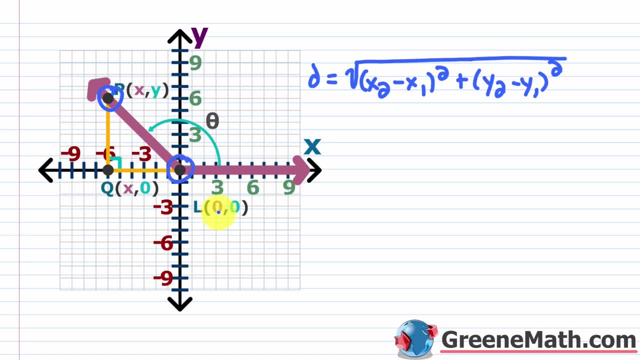 the point O. okay, for origin. I'm just going to call it the point L because I don't want you to get confused with coordinates there: zero and zero, okay, It looks too similar. So point L here. zero, comma zero is my origin. I also have another point here to form a right triangle. okay, which? 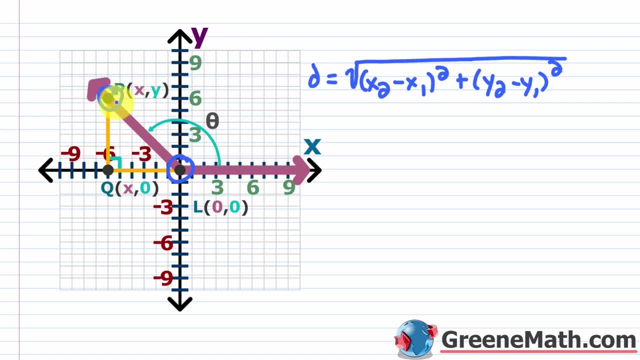 is point Q which has the coordinates x- right because it's got the same x location, and then zero- right because it's on the x axis. So x comma zero. So we can see that we can form a right triangle and obviously you could use the. 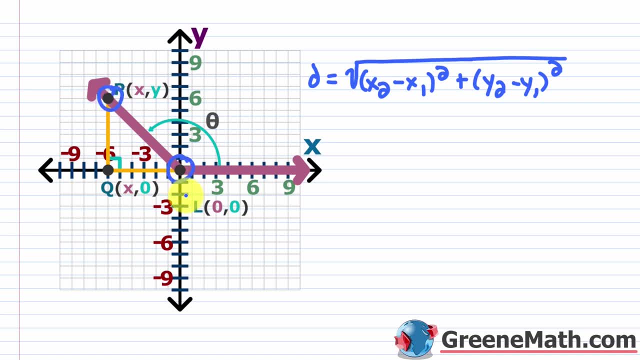 Pythagorean formula to find the distance from point P to point L, or the origin, or you could just plug into the distance formula, which is much easier. Now, what we're going to do is we're going to replace the D with an R. okay, and I'll explain why that occurs in a future lesson. Let's 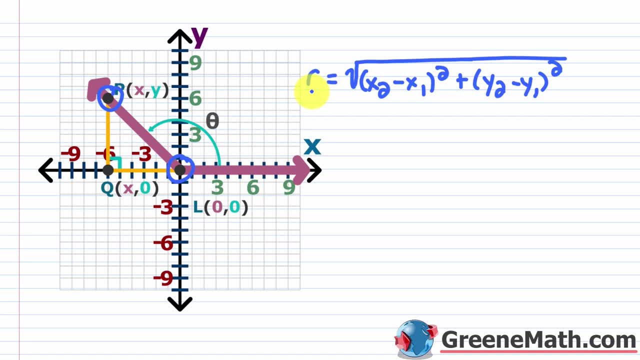 get to the unit circle first. I want to just keep this simple. Additionally, since we're working with a point that is zero comma zero, I can replace this with a zero and this with a zero. okay, and now I no longer have an x sub 1 and an x sub 2, or y sub 1 and a y sub 2,, so I can just. 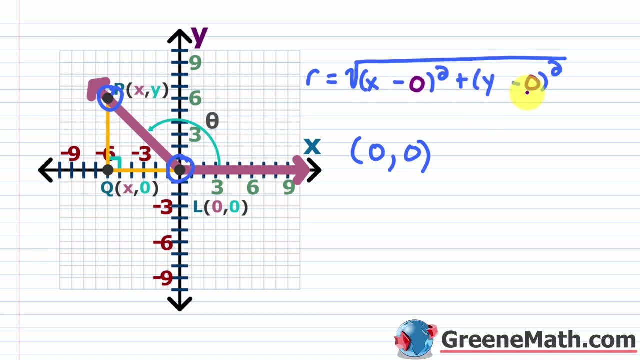 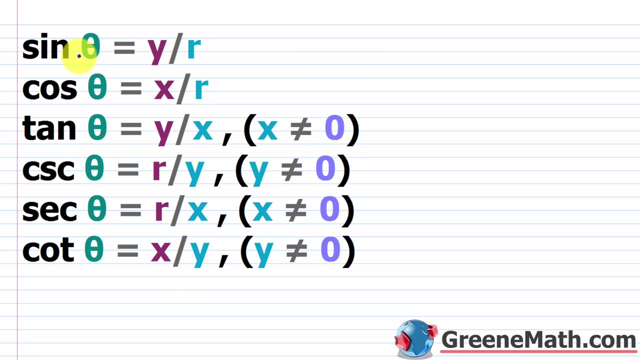 drop this notation. okay. We know that x minus zero is x and y minus zero is y, so I can just really say this is x squared okay plus y squared under this radical, okay. So we've made that quite simple now in terms of the definition for R. All right, so let's take a look at the six trigonometric. 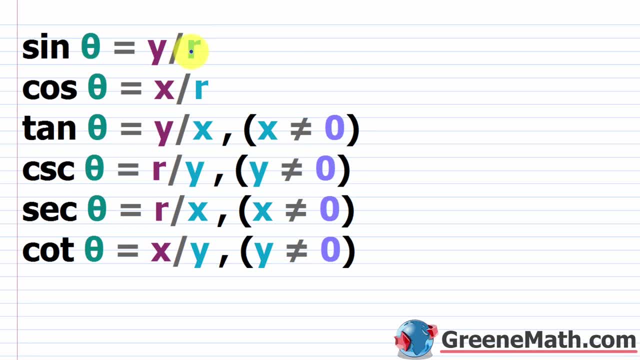 functions that we're going to work with. Remember this R here that you see in these formulas refers to what I just wrote. It's the square root of x squared plus y squared. Now, as we move forward in the course, we'll see different ways to remember this. I know a lot of you think about. 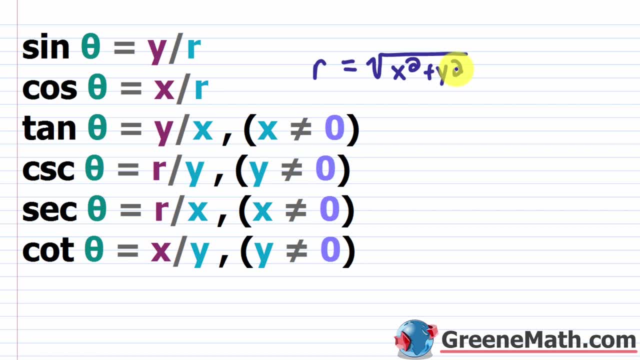 the SOHCAH TOA. okay if you've taken trigonometry before, but for right now we're just going to keep this really, really simple. We'll get to that later on. So the sine of theta is going to be. 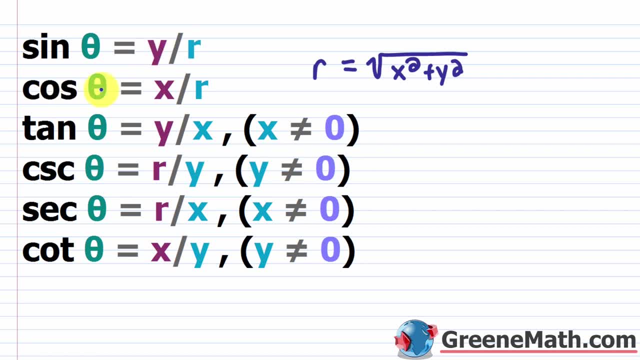 equal to y over R, Then the cosine of theta is going to be equal to x over R. Then the tangent of theta is going to be equal to y over x. where x is not equal to zero. The cosecant of theta is going to be equal to R over y, where again y is not equal to zero. The 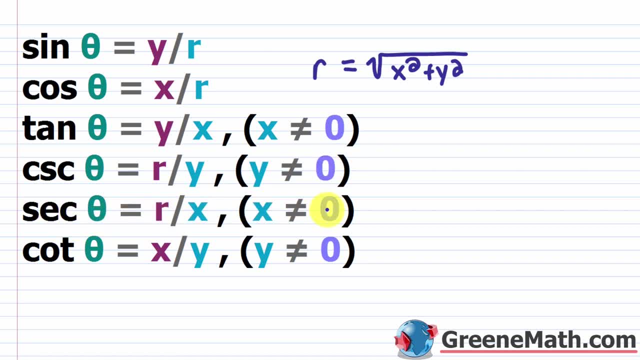 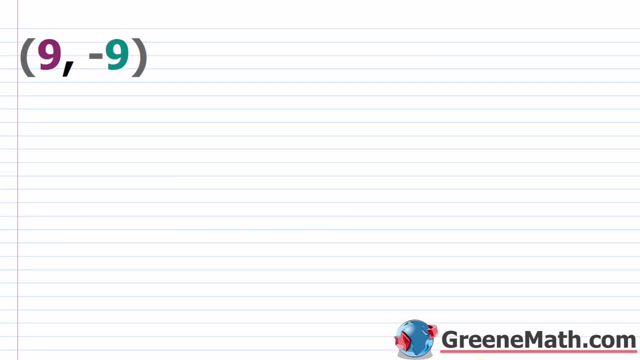 secant of theta is going to be equal to R over x, where x is not equal to zero, And the cotangent of theta is going to be equal to x over y, where y is not equal to zero. All right, so let's go ahead. 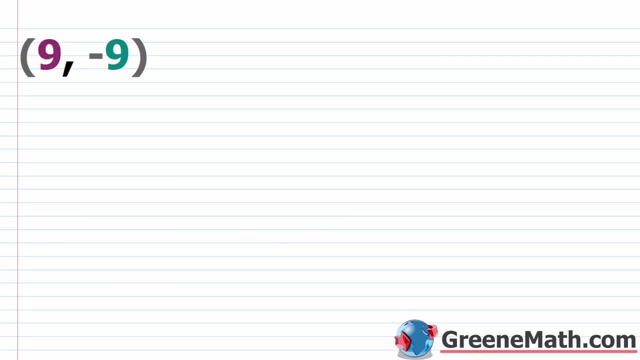 and look at an example. Let's say that we're given the point nine comma negative nine And basically it's going to be the terminal side of the angle. theta in standard position is going to pass through theta Again, nine comma negative nine would be the coordinates And we want to find the values of. 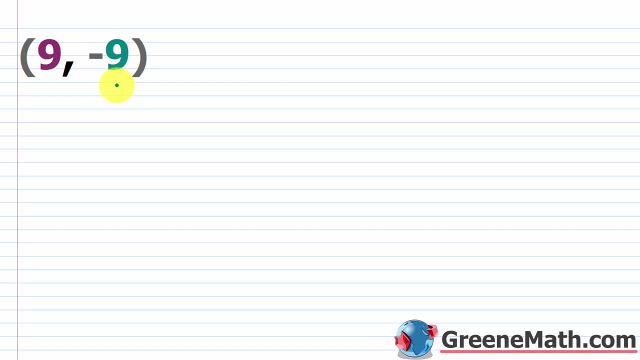 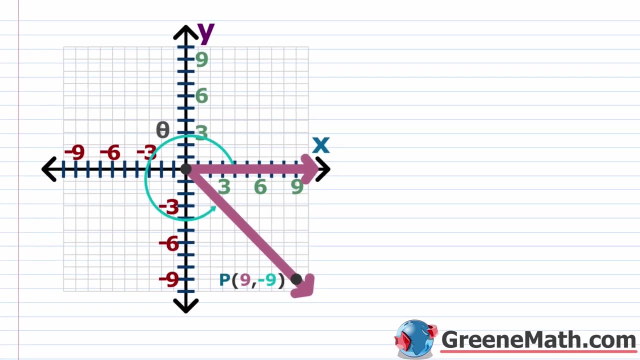 the six trig functions here. So let's do a quick sketch. A lot of people like to do that to see what's going on. It's not completely necessary because you're just going to be plugging some things in, but just to get an idea of what's going on. So if we highlight this point here, 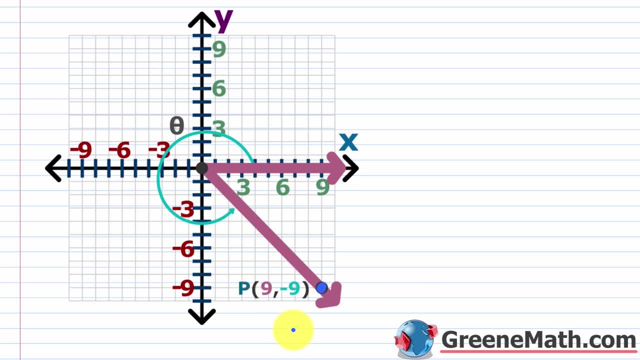 again, this is nine comma negative nine. That's going to be our point. Let's just call it P, okay, And basically what we're looking at is our angle here, theta. okay, So we want to find the six trigonometric functions based on this guy. 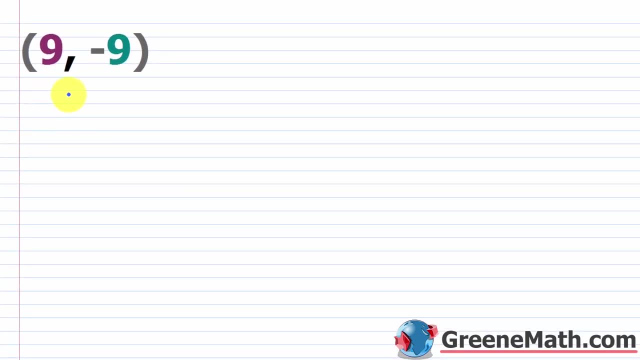 So let's go back up and let's remember that this is our x value. So our x value is going to be nine. Our y value is going to be negative nine. Just pull it straight from this ordered pair here. okay, So this is your x and this is your y. okay, Make sure you bring the signs along for the ride. 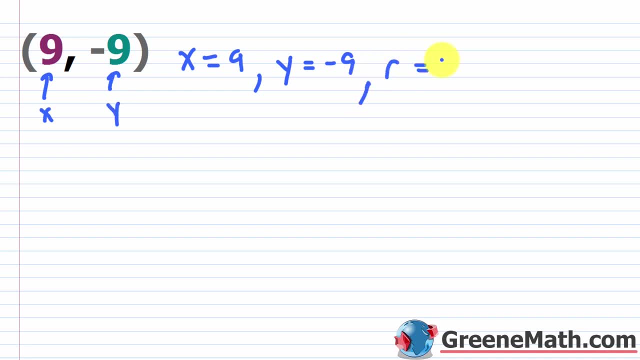 Then your r value is what? Remember? this is found by taking the square root of x squared plus y squared. So the square root of x squared, x is nine, nine squared is 81, y squared, Y is negative nine. Negative nine squared is also 81. So you could really write: 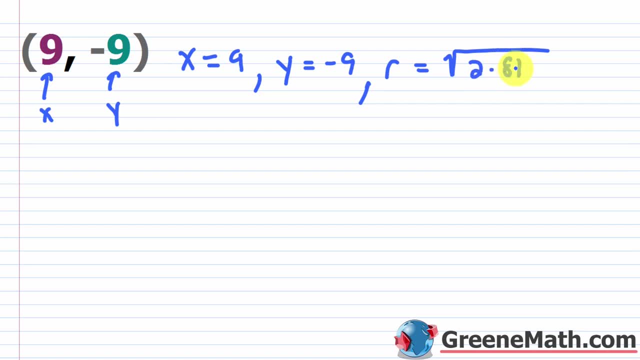 this as two times 81 to make it a little bit cleaner. okay, Because you know that 81 is a perfect square. The square root of 81 is nine, So you could really say this is nine times the square root of two. To find all the trigonometric functions, you're just going to plug in what? 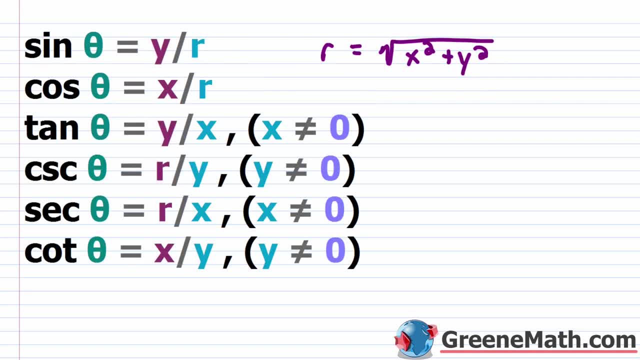 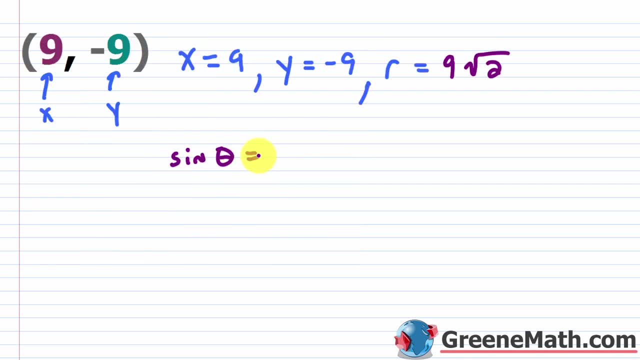 theta, sine of theta is y, okay, which is negative, nine over r, which is nine times the square root of two. Okay, Well, we know we want to rationalize this denominator. First off, we can simplify this, because this would be negative one, But we want to rationalize this, So let's multiply the numerator. 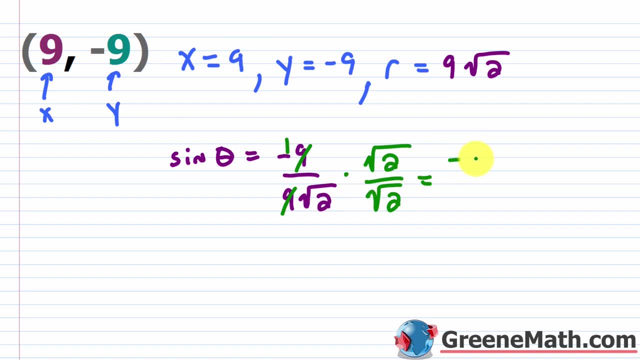 and denominator by the square root of two, And this would give us what It would give: a negative square root of two over two. okay, So that would be your sine of theta. So let's erase this and just kind of make this a little bit. 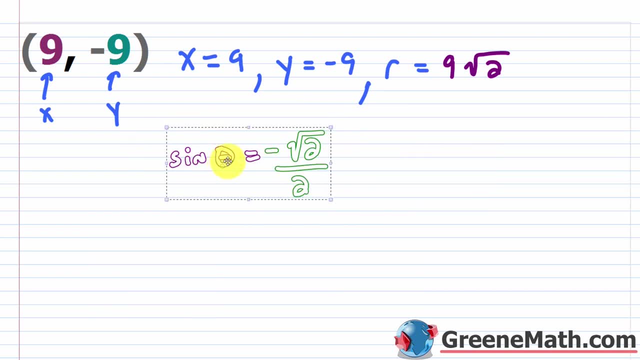 cleaner. Okay, So we'll bring this down and bring this a little bit over, And so now let's look at the cosine of theta. So this is x over r. So the cosine of theta, okay, So this is x over r. 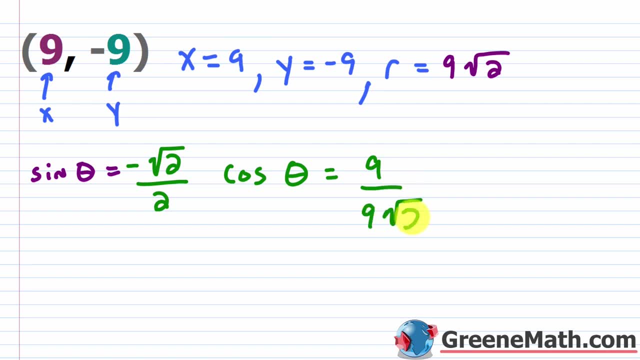 x is nine And again r is nine times square root of two, And basically you're going to get the same thing as this. When you rationalize, it'll just be positive. okay, So you would cancel this with this and get a one here, And you'd multiply the numerator and denominator by the square root. 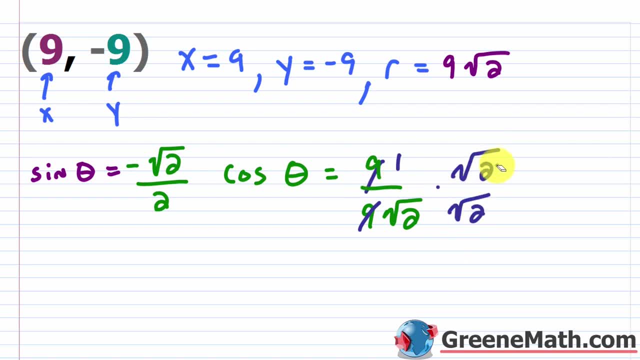 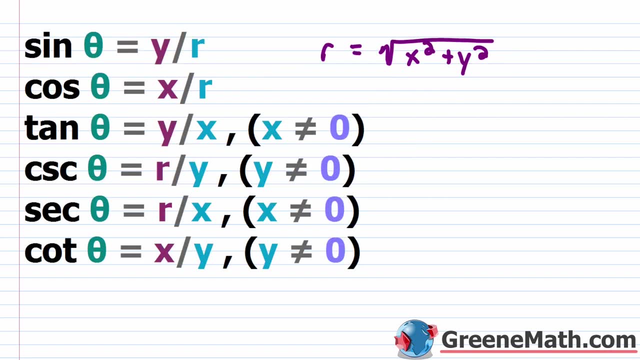 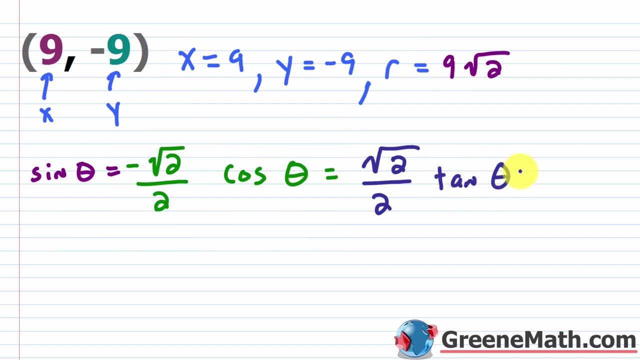 of two And essentially you would have what You'd have: the square root of two over two. So this is the square root of two over two, Okay, So the next one is the tangent of theta. okay, So y over x, So the tangent of theta, okay. So what is y That's negative? nine, What is x That's positive? 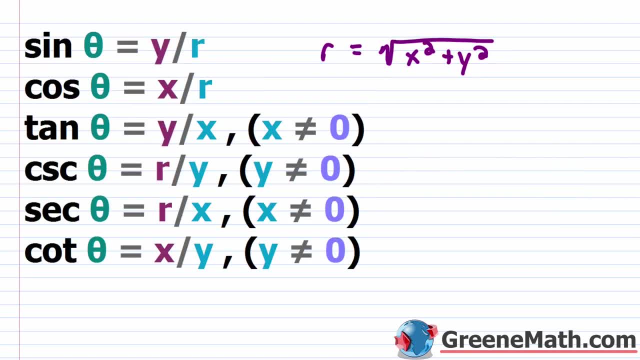 nine, So that would be negative one, All right. So next we have these guys that we can find by flipping things. okay, So So we know that the cosecant of theta can be found by flipping the sine of theta. okay, Because this? 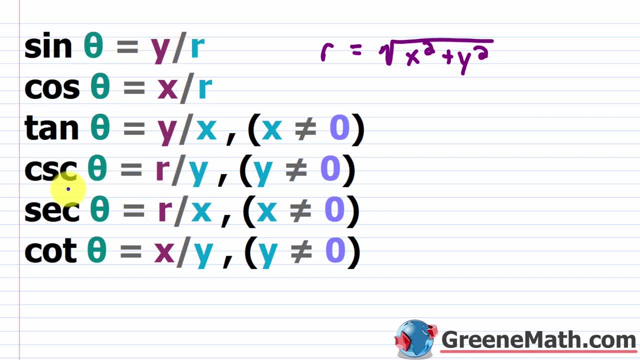 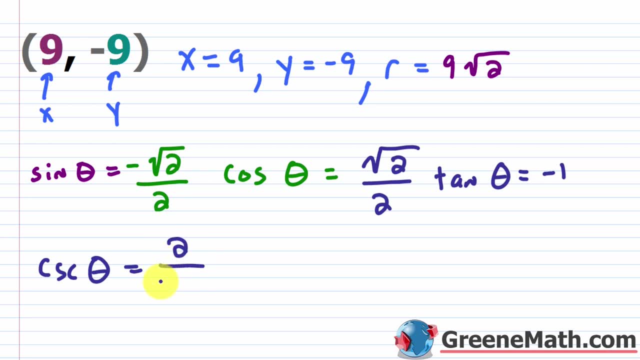 is r over y. this is y over r. So all I want to do for the cosecant of theta is just flip this guy. okay, So I would have two over the negative square root of two And, if you're smart, before you. 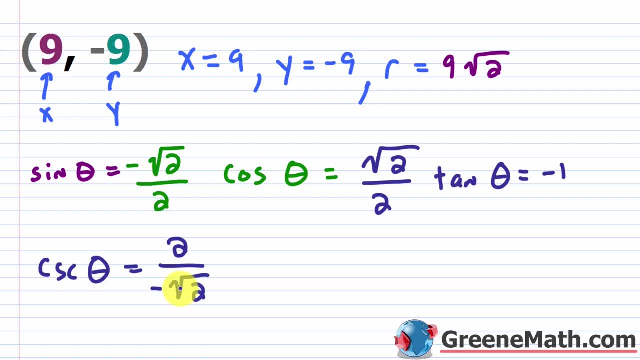 rationalize that guy. you'll go ahead and flip it right, Because now we have to rationalize again. So I'm going to multiply this by the square root of two over the square root of two And that would be negative out in front. two times the square root of two over this would be two And you can. 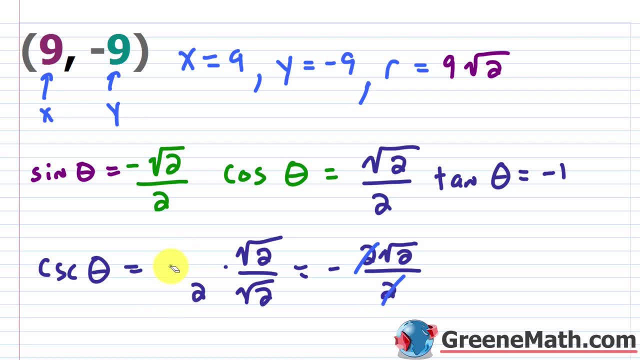 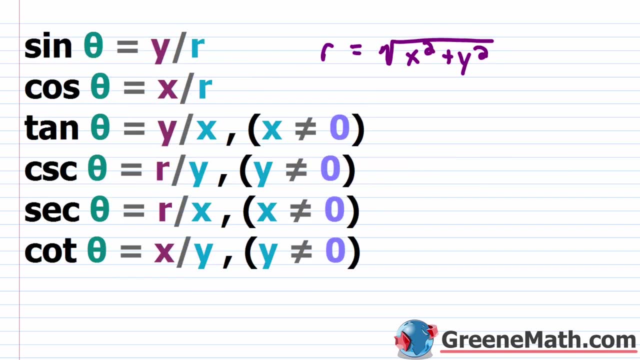 cancel this would cancel with this, and you're just left with the negative square root of two. okay, So the negative, the negative square root of two. So then we go back and we see that the secant of theta is r over x. So I'm just flipping the cosine of theta, So I'm just flipping the. 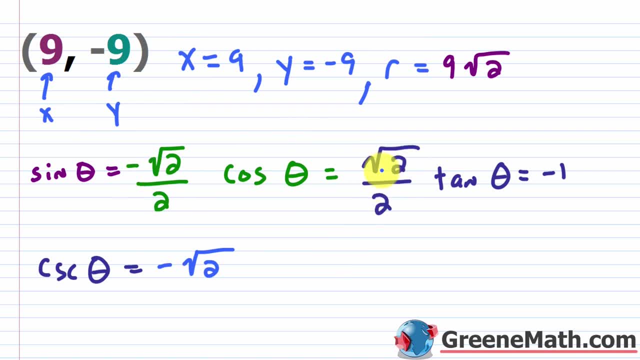 cosine of theta. And again, the only thing that was different between this one and this was the sine. So I know that the secant of theta is r over x, So I'm just flipping the cosine of theta. Okay, the secant of theta is going to be equal to the square root of two. Again, you can go through. 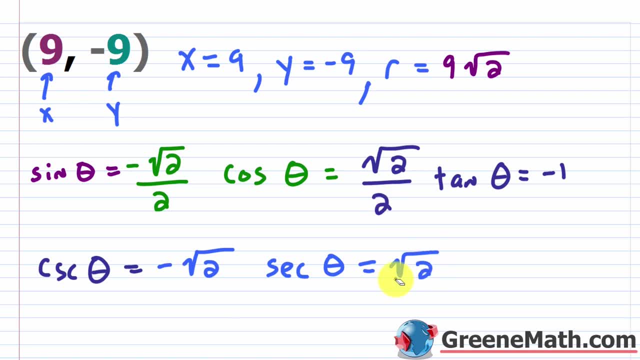 this on your own. you would flip this- and let's just do it real quick so that nobody's confused: It's two over the square root of two. you multiply this by the square root of two over the square root of two, And so what do you get? You get a two down here. okay, that's going to now cancel. 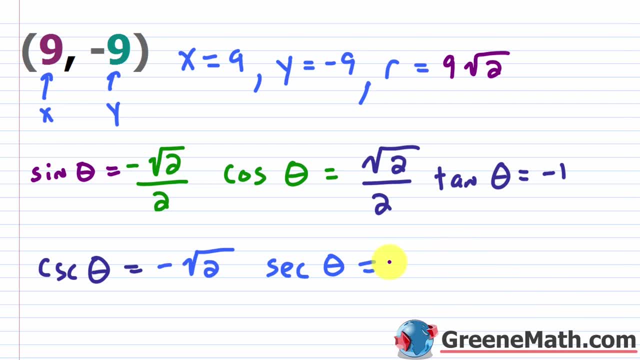 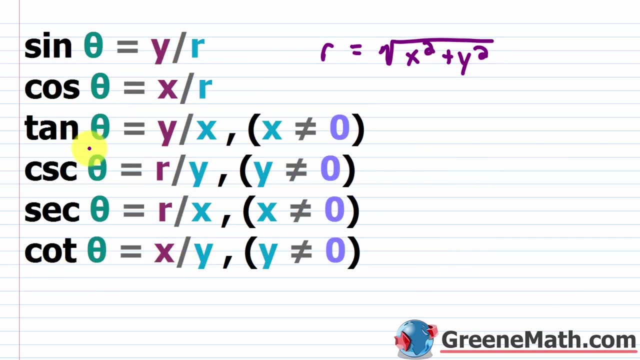 with this two up here, you're left with just square root of two. okay, So that's how we got that. Now, the last one is the cotangent of theta, And that is found by flipping the tangent of theta. okay, In this case, the tangent of theta was negative one. So if you think 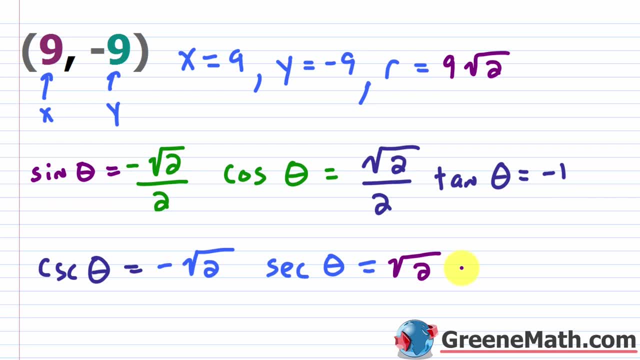 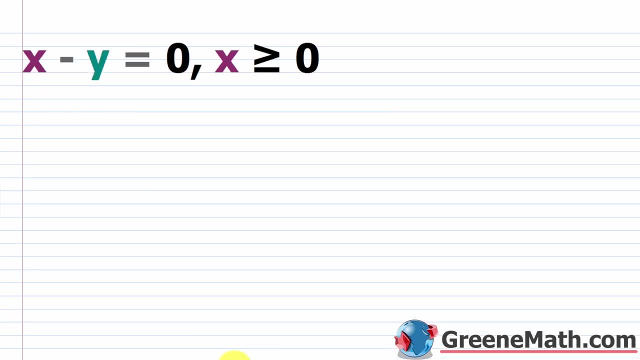 about it. you really say that's negative one over one. flip it, you still have one over negative one, which is still negative one. So my cotangent of theta will be negative one as well. All right, so let's look at another example. We're going to change things up just a little bit. 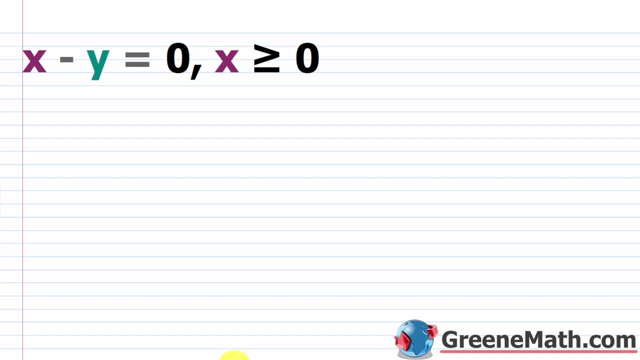 So you might also be asked to find the trigonometric function values of an angle when we know the equation of the line that coincides with the terminal ray. So I want you to think for a second. we all know that the equation of a line in standard form, 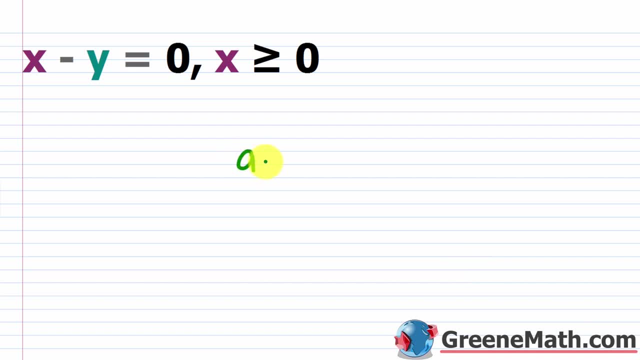 that passes through the origin looks like this: So it's something ax plus by equals zero. So, for example, this x minus y equals zero. if I didn't consider this restriction, that would be a line that passes through the origin okay, But what we're going to do here is we're going to restrict. 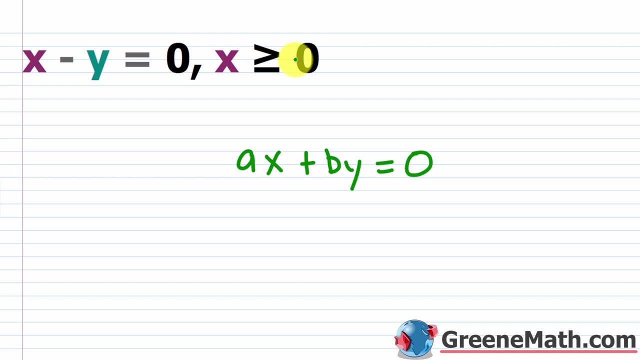 the x values to either be x is less than or equal to zero, or x is greater than or equal to zero. okay, What we're going to get is a ray with an endpoint at the origin. okay, So let's look at an example of this down here, okay, And 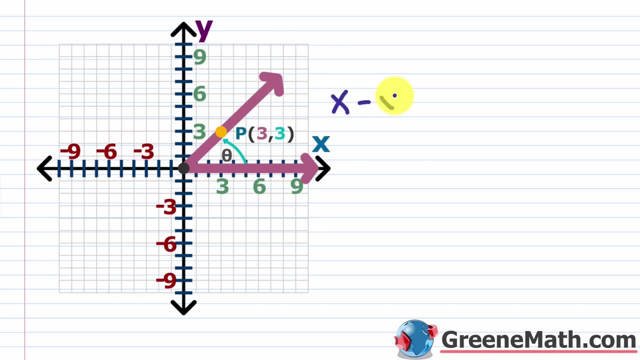 what you see is that we have x minus y is equal to zero. okay, That line would be drawn if I extended it past this point. Let me kind of highlight this in a different color If I extended it past this point: zero, comma zero. But we're going to restrict the x values to be greater. 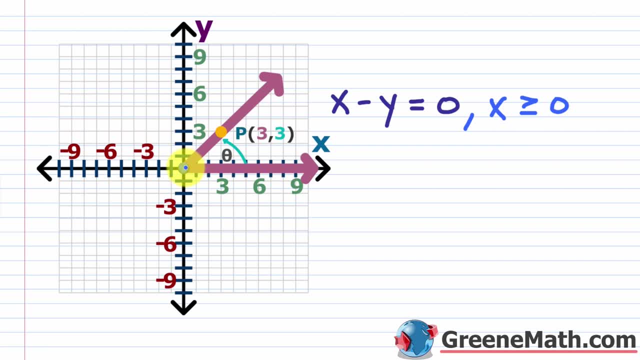 than or equal to zero. So we're only going this way. So this is the endpoint and we go this way. So this is your terminal, okay, So you might see this as well. All you need to do is pick a point. That's not the origin. So 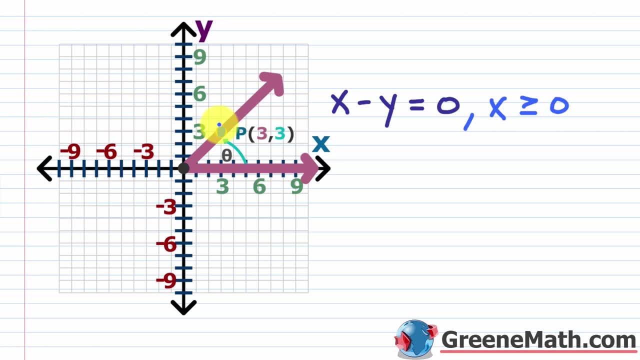 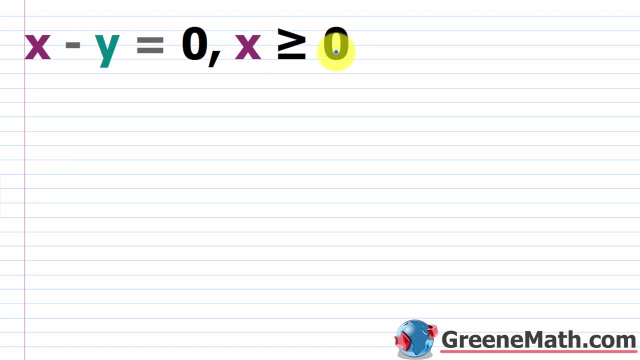 in this case I've picked the point three comma three. okay, And one way you can do that: if you haven't drawn this guy, you can just pick an x value that lies in this range. Again, don't pick zero. So let's say you chose three, Plug in a three for x. So you know that x is three Solve. 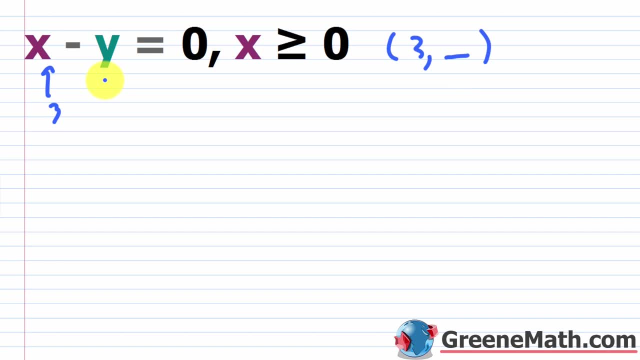 for the unknown y. What's it going to be In this case? you can eyeball it and see it's going to be three as well. But again, if you had to solve, you would just say: okay, three minus y equals zero. 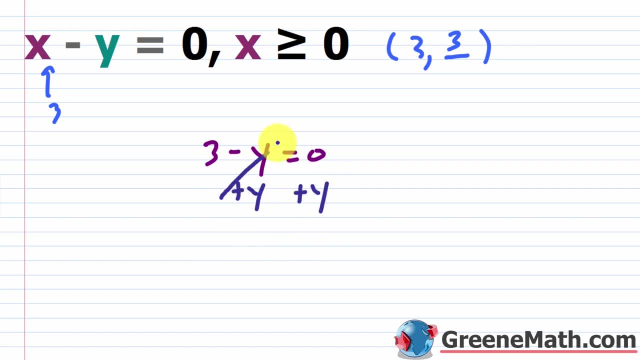 Let me go ahead and add y to both sides of the equation And this would cancel and I get three is equal to y. Okay, so x is three, y is three. This is going to make it really easy for us to crank out those. 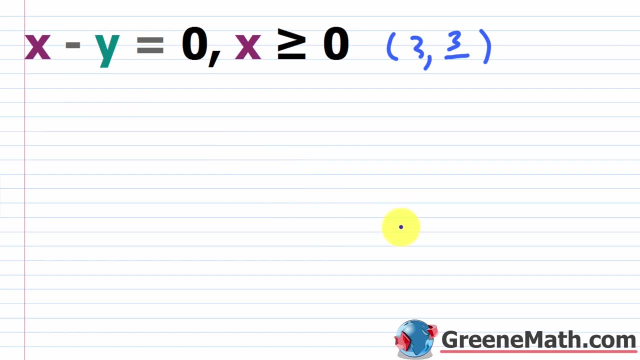 six trigonometric functions. So what I'm going to do here is go through them more quickly. So let's just write them out. So we have sine of theta, And this is equal to our y value over our r value, And we'll get r in a minute. Then we have our cosine of theta. Okay, so this guy is going to 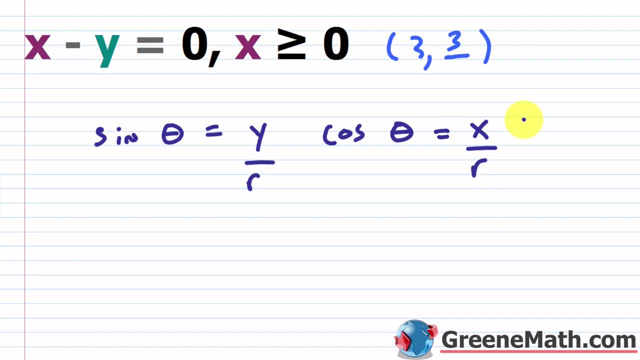 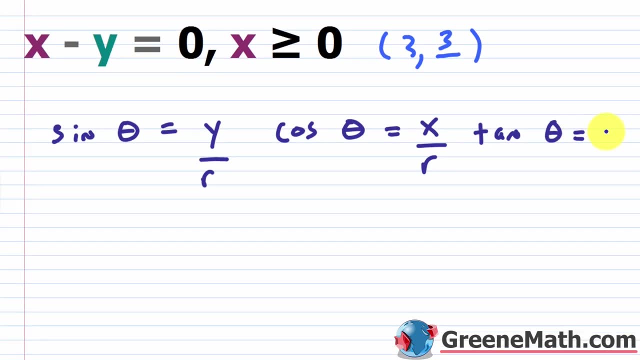 be the x over the r. Okay, then you have the cosine of theta. So this guy is going to be the cosine of theta, And then you have your. let me slide this down a little bit, So we're a little too far over. So we have the tangent of theta. This is going to be equal to your y over your x. 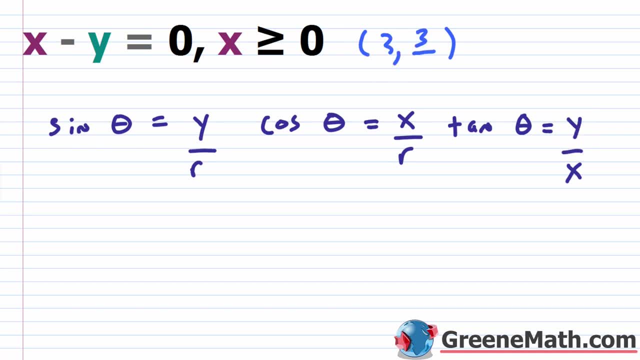 Now we can crank this one out right now, because x is three and y is three. Let me label this: This is x, This is y, So three over three, we know would be one, So let's just put that down right now. Okay, then we know that the cosecant of theta- okay, the cosecant of theta is found by 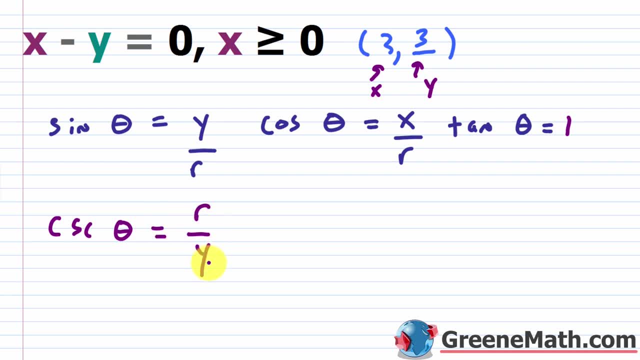 just flipping this guy, So it's going to be r over y. Then the secant of theta is going to be r over y. Okay, the secant of theta is found by flipping this guy, So it's r over x. And then the cotangent. 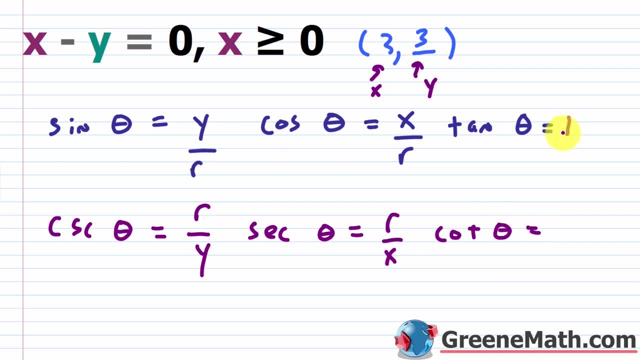 of theta is found by flipping this guy. In this case, you flip one, right, If you had one over one and you flipped it, you still have one over one, So it's just one. So what is r in this case? 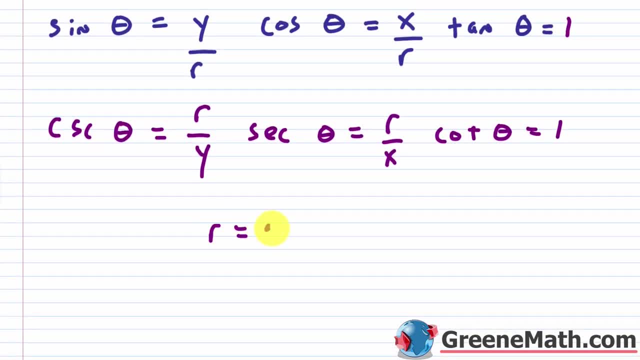 Well you would have. let's scroll down and get some room going. So r is equal to the square root of x squared plus y squared. Okay, so x is three, y is three, Three squared is nine. So you'd have. 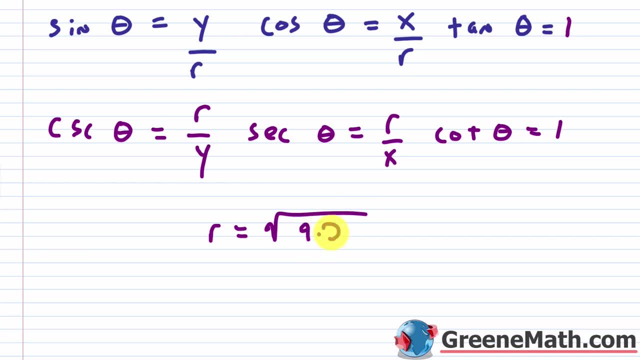 nine plus nine or 18, right. So 18 is nine times two. Nine is a perfect square. It's three times three. So pull that out and you'd say this is three times the square root of two. Okay, so what I'll do is: everywhere there's an. 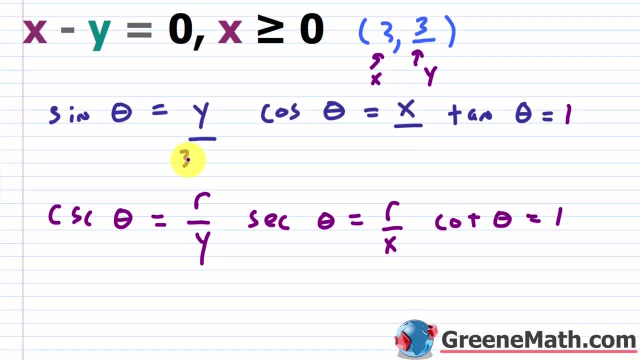 r. I'll just replace it with three times square root of two, So three times square root of two and three times square root of two, And you can do it here as well. But what's going to happen is we're going to crank these out really quickly, because these are going to be the same and these 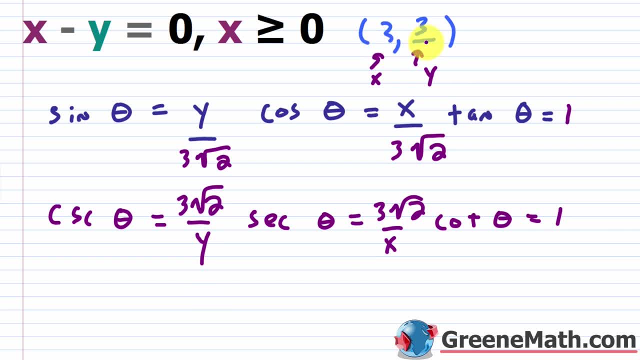 are going to be the same. Okay, because we have the same x and y value, So x and y, as I just said, are the same. So I'm going to put a three here and a three here And you can put a. 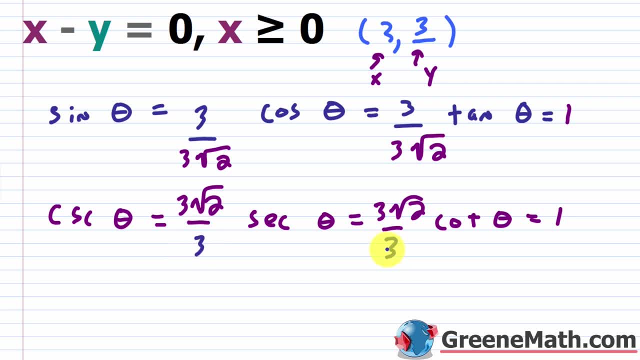 three here and a three here. Okay, And very quickly, we can see that this cancels and this cancels. So this is going to be the square root of two in each case. Okay, And we can write that more cleanly: square root of two. And let's write that more cleanly: square root of two. 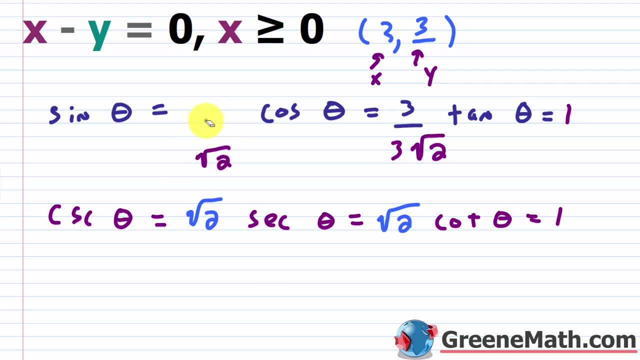 And in this case we need to rationalize, right. So we'd have one over the square root of two. And if I multiply by the square root of two over the square root of two, well, down here I would have two, Okay, And up here I would have the square root of two. So 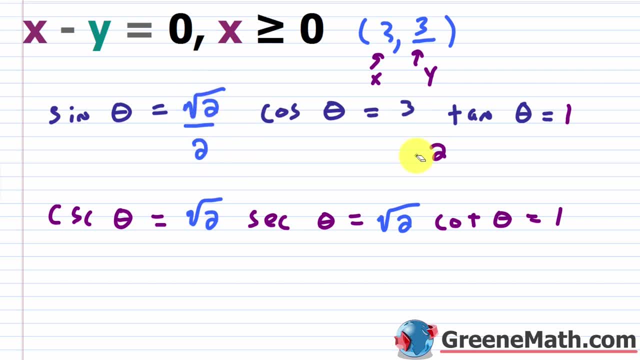 let's write this as the square root of two over two, And this is the same right. So this is the square root of two over two, All right, So these were more simple examples. As we progress, we'll see things that are much more challenging. In this lesson, we want to talk about reciprocal 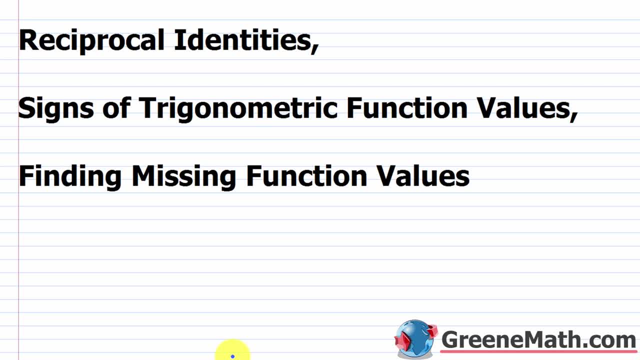 identities, signs of trigonometric function values and also how to find missing function values when we're given one value in the quadrant of the angle. All right, So let's begin our lesson by talking about the reciprocal identities. So in the last 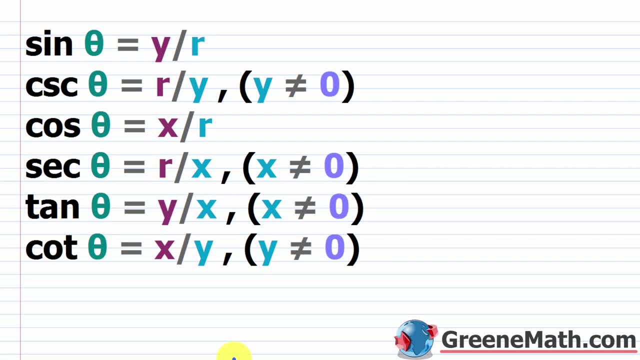 section we talked about the six trigonometric functions. We found that some of these functions are reciprocals of each other, So keep in mind when we use the value of r. okay, r, by definition, is equal to the square root of x squared plus y squared. Okay, And we talked about that in the 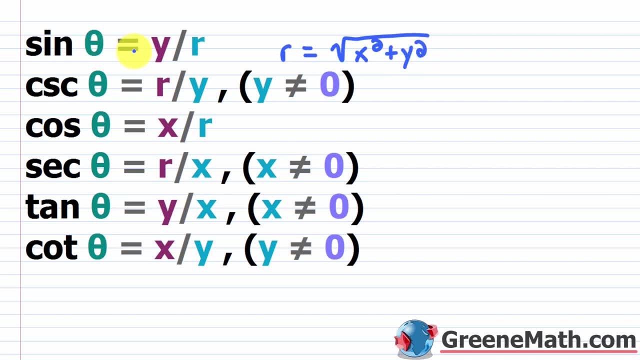 last video. So we see that sine of theta is equal to y Divided by r. Okay, And then cosecant of theta is equal to r divided by y, And then in this case, y is not equal to zero. We don't have to have that restriction for r there, because r is always. 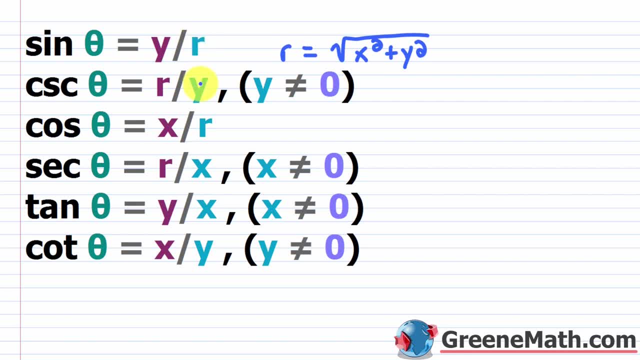 going to be a positive number, Okay, But we do need it here because y could be zero. So these guys, the sine of theta and the cosecant of theta, are reciprocals. So if you know one, you automatically know the other by just flipping the fraction. Okay. And then the same thing goes when. 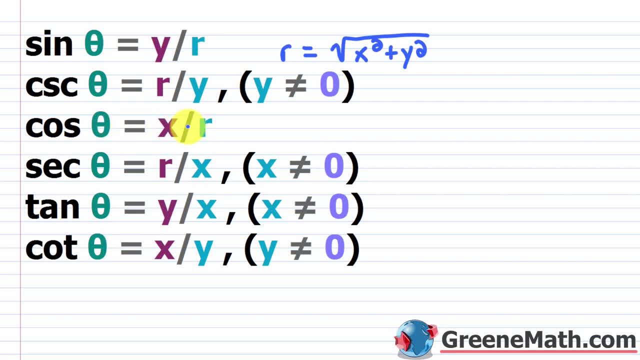 we look at cosine of theta, which is x over r, And secant of theta, which is r over x, Again, x is not equal to zero here. Then again, when we look at the tangent of theta which is y over x, x is not zero And the cotangent of theta, which is x. 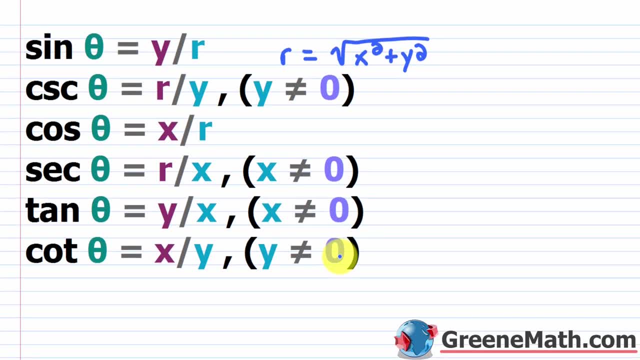 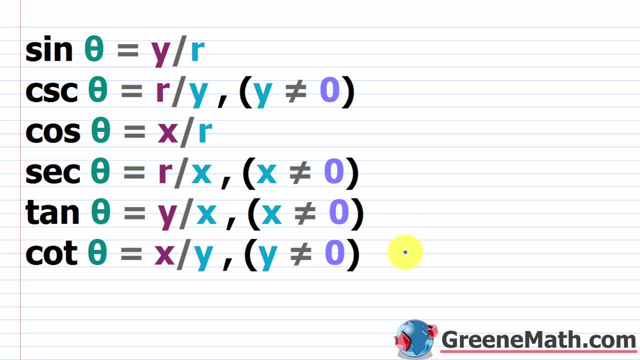 over y, y is not equal to zero. Those guys are reciprocals of each other as well. So in your book, when you're talking about the reciprocal identities- let me erase this real quick- They'll write them in a specific way So we can say that the sine of theta okay is equal to one. 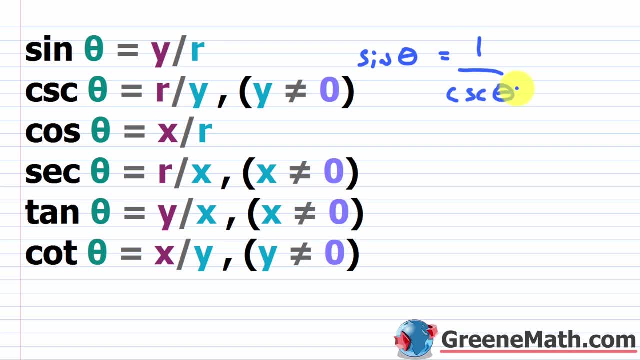 secant of theta. Okay, Then you could also say: the cosecant of theta is equal to one over the sine of theta. Remember, if you have one divided by something, okay, all you're doing is you're ending up taking the reciprocal. So if I had one divided by one divided by y over r, you could. 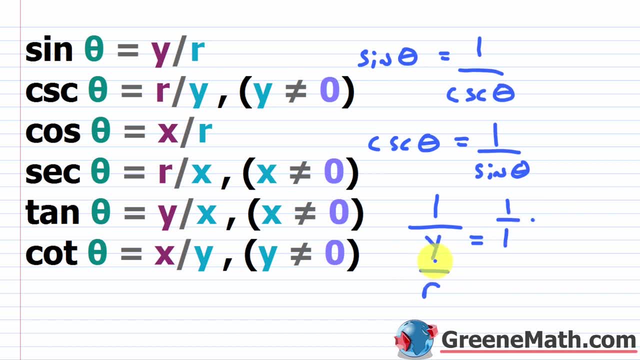 really say: this is one over, one times the reciprocal of this guy, So r over y. So this ends up being r over y. Okay, So that's all that is. It's just fancy notation. So let's erase this real quick and let's keep going So we have the sine of theta is one over. 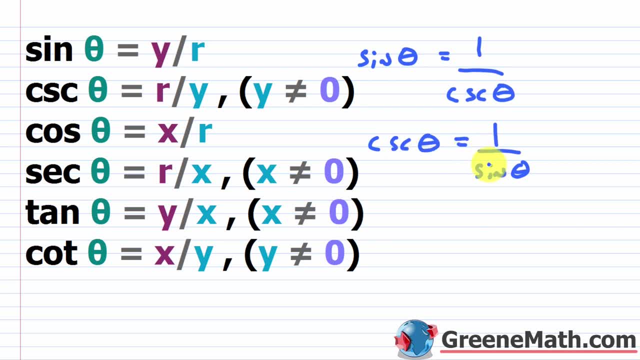 the cosecant of theta. The cosecant of theta is one over the sine of theta. Then you say the cosine of theta is equal to one over the secant of theta. Okay, And then the secant of theta again, it's just one over the cosine of theta. Let's write these down here. So the tangent of 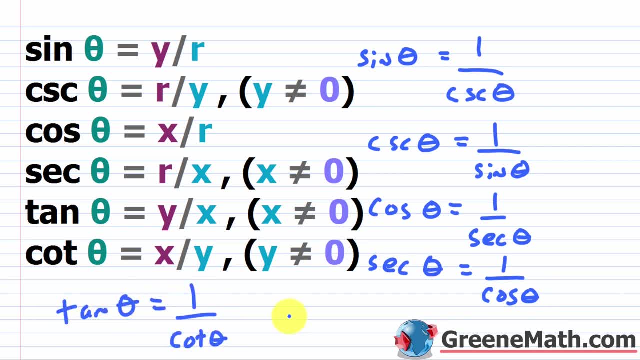 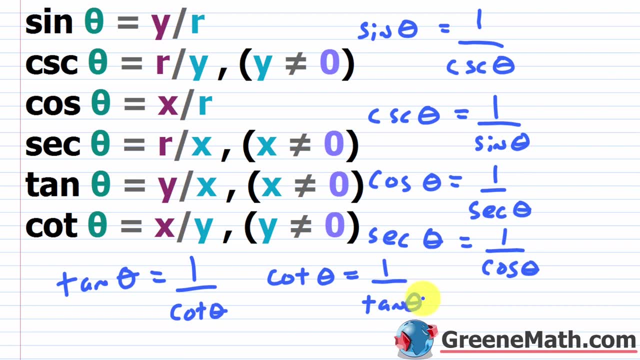 theta is equal to one over the cotangent of theta And, of course, lastly, the cotangent of theta is going to be equal to one over the tangent of theta. Okay, So that's all this is. It's not very complicated when you see this in your book. the topic of reciprocal 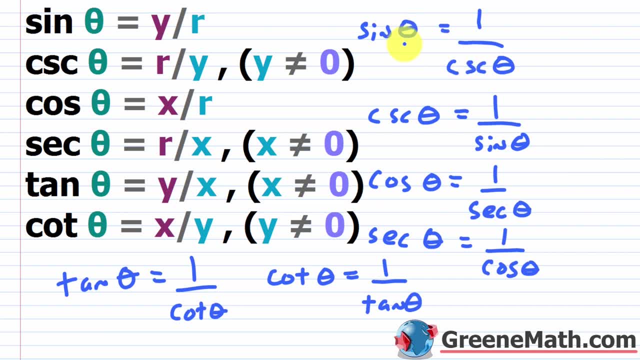 identities. You take the two guys that are reciprocals. Okay, One will be over here, One will be in the denominator. You can switch the positions Again: the sine of theta and the cosecant of theta. those guys are reciprocals, So the sine of theta is equal to one over the. 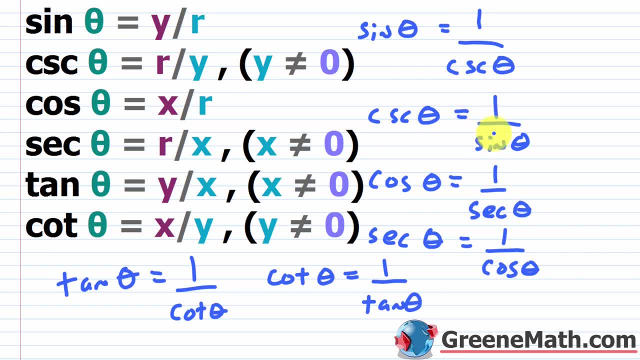 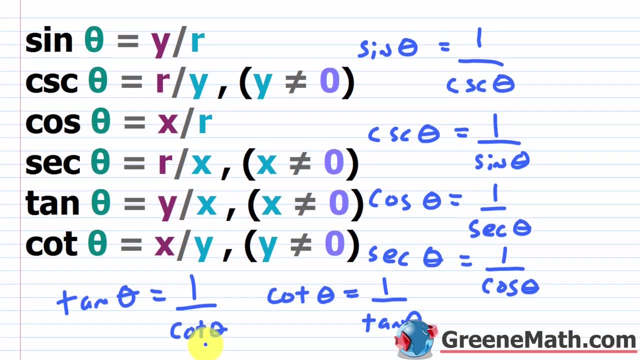 cosecant of theta. Similarly, the cosecant of theta is equal to one over the sine of theta. You see the same thing with the cosine of theta and the secant of theta and with the tangent of theta and the cotangent of theta. So let's look at a quick. 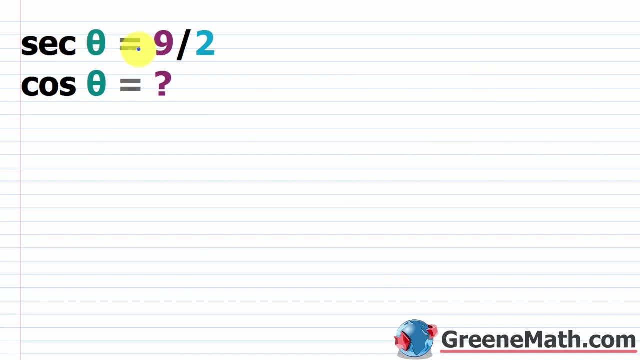 example of this. So we have that the secant of theta is equal to nine halves, or nine over two. What is the cosine of theta? Well, again, the secant of theta and the cosine of theta. those guys are reciprocals of each other. So if this guy is nine halves, all I have to do is flip. 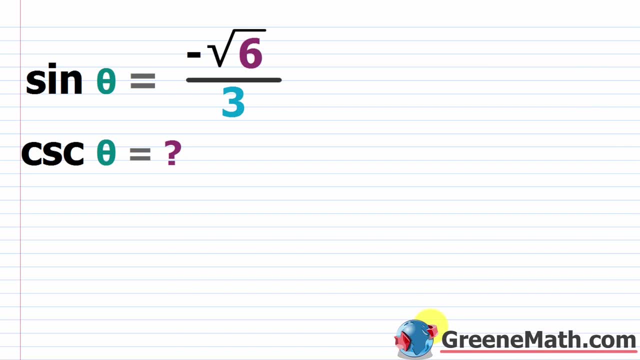 it and it would give me two ninths. All right, let's take a look at another example. So here we have: the sine of theta is equal to the negative of the square root of six over three. What's the cosecant of theta? Again, these guys are reciprocals, So I can just flip them and say: 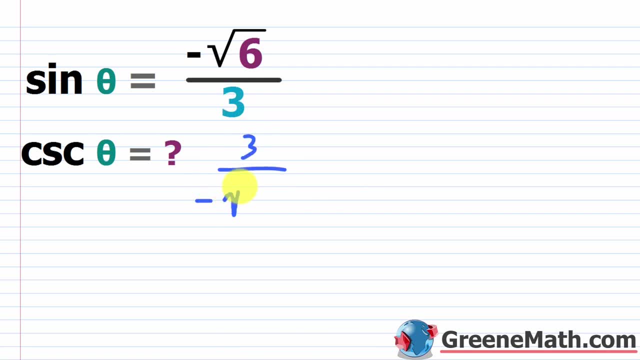 this is three over the negative square root of six. Okay, what I'm going to do is I'm just going to put my negative out in front And then I'm going to multiply the numerator denominator by the square root of six, So I can rationalize the denominator. So this will be equal to the negative. 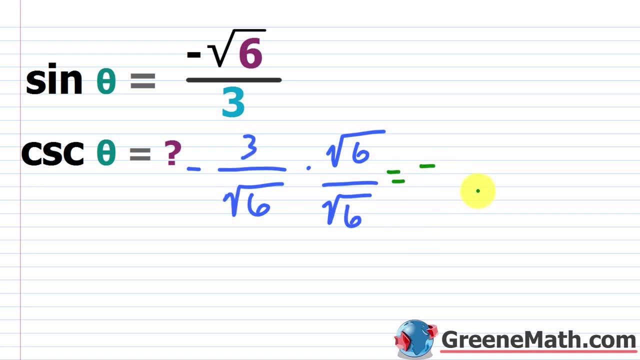 of, we'll have square root of six times square root of six is going to be six And you'll have three times square root of six up here in the numerator. Of course you can cancel. This would cancel with this Which is divisible by three, So this would just be one, So you can just get rid of it And six. 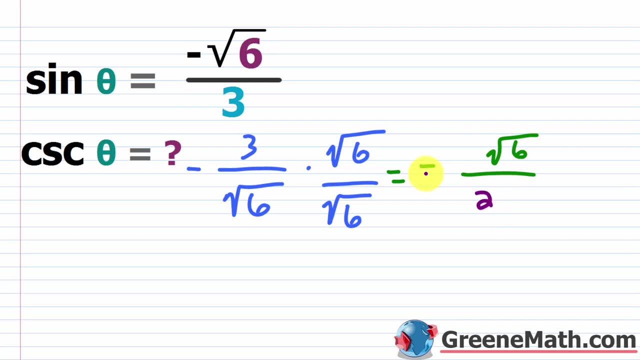 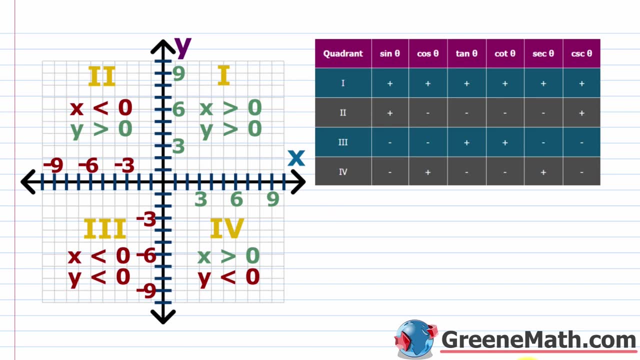 divided by three is two. So your final answer here would be the negative of the square root of six over two. All right, let's talk about the signs of the trigonometric function values. So we know that when we defined the trigonometric functions, we gave r as the distance from the 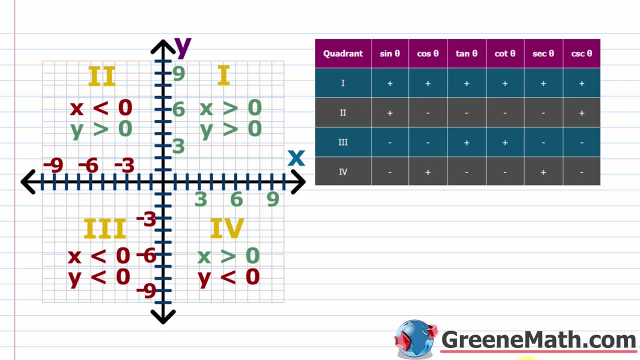 origin, or the point zero, comma zero, to the point x comma y. So, since this distance is going to be undirected, okay, the value of r is always going to be positive. So if you look at something like sine of theta, okay, we know that this is defined as y over r. 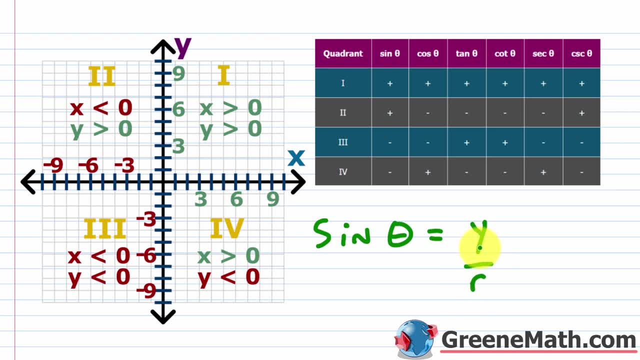 okay. So since r is always positive, we think about the sign coming from just whether or not y is positive or negative. So if you look at your coordinate plane, remember there's four quadrants. In the first quadrant you have the x and y values that are positive. In the second quadrant, 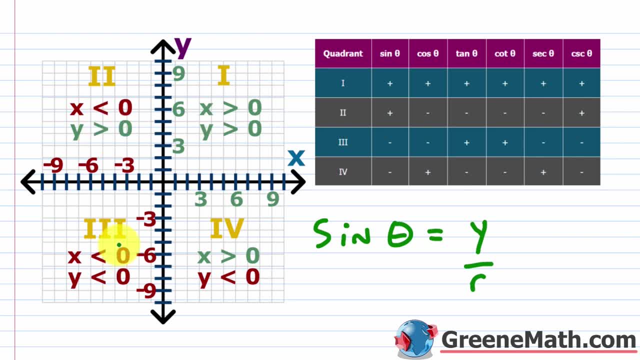 the x values are negative. the y values are positive. In the third quadrant, both the x and y values are negative. In the third quadrant, both the x and y values are negative. In the third quadrant, both the x and y values are positive. and in the fourth quadrant, the x value is positive. 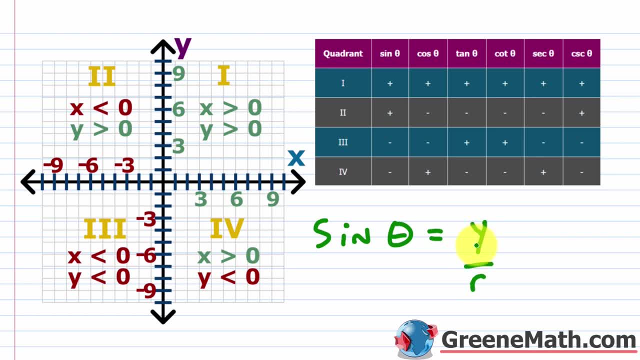 the y value is negative. okay, So where is y negative? It's negative in quadrants three and four. So that means if I'm in quadrant three or four, the sine of theta is going to be negative, because r is always positive. right, You would end up with a negative over a positive, which gives me 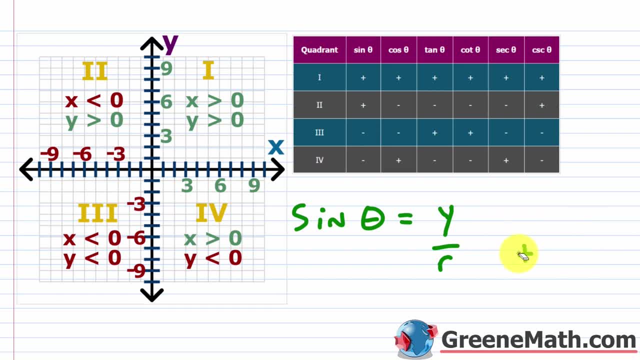 a negative. okay, And I should have put a negative there, But if you look at this little table I have up here, this summarizes everything for you. In the first quadrant, where x and y values are positive, trigonometric functions are positive. In the second quadrant, where x is less than zero and y 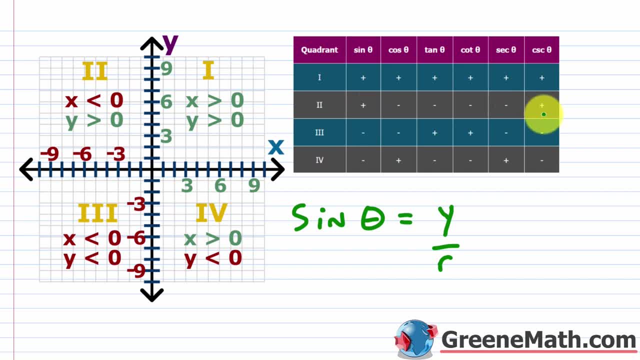 is greater than zero, your sine of theta is going to be positive, and then the reciprocal, the cosecant of theta, is going to be positive as well. As we move into the third quadrant, where again x and y values are both negative, you get just that tangent of theta and cotangent of theta- Again those guys. 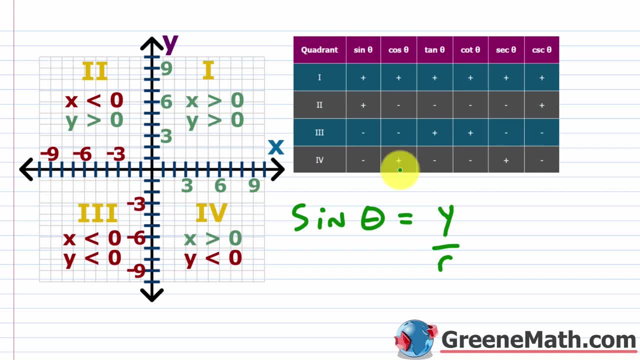 are reciprocals. Those guys are positive, everything else is negative. And then in the fourth quadrant, where x values are positive and y values are negative, you'll see the cosine of theta and also cosine of theta. Again, those guys are reciprocals. Those guys are positive, everything else is. 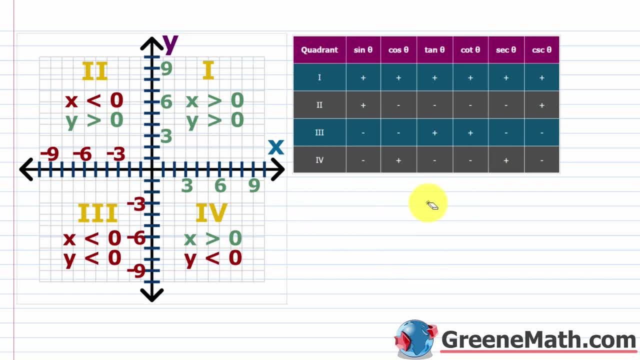 negative. So an easy way to remember this, because trying to remember this chart is kind of hard, is a little mnemonic device. All students take calculus. okay, So just take the first letter from each. So all a students s take t and c for calculus. So all students take calculus and this goes. 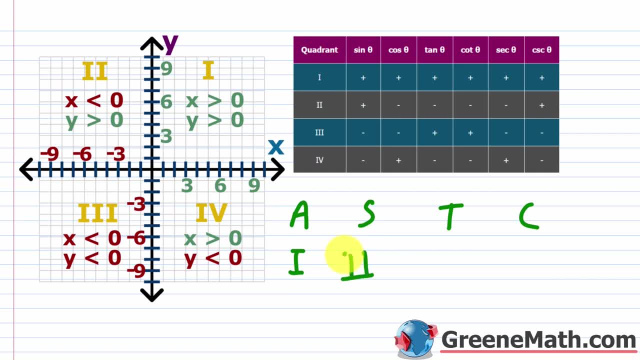 counterclockwise. So this is for quadrant one, this is for quadrant two, this is for quadrant three and this is for quadrant four. okay, So the a is for quadrant four and this is for quadrant five. The a just stands for all. so all six trigonometric functions in quadrant one are going to be: 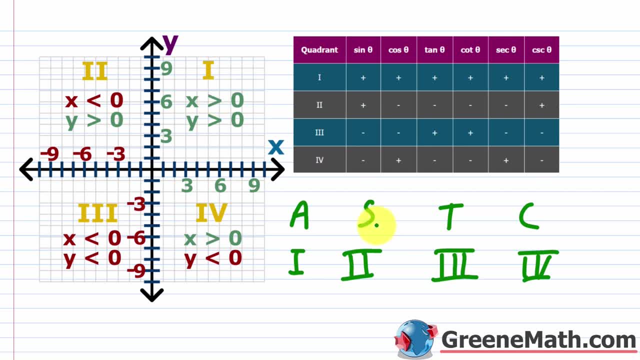 positive. The s is for sine, okay, So the sine of theta, okay, is going to be positive and you know the reciprocal of that will be positive as well. The reciprocal of the sine of theta is going to be the cosecant of theta. So sine of theta and cosecant of theta are positive in quadrant two, Then in: 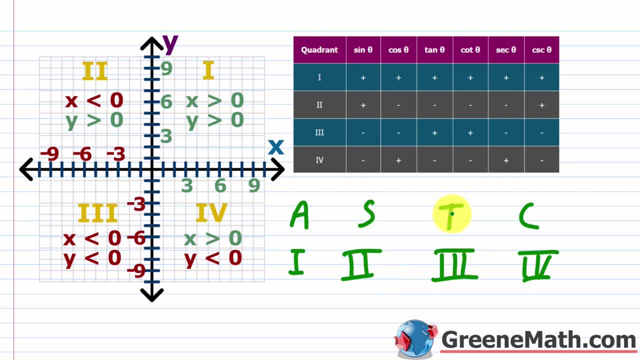 quadrant three, you have t for tangent of theta and then also the reciprocal, the cotangent of theta. So those guys are positive, everything else is negative. And then in the fourth quadrant you have a c for cosine of theta and the reciprocal of that is the secant of theta. So again those two. 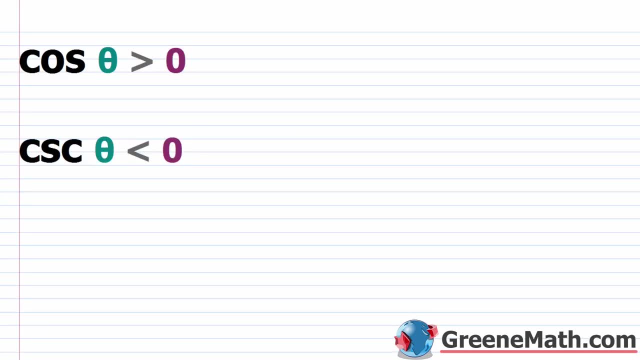 are positive. everything else is negative. All right, so let's use what we just learned to look at a few examples. We're going to identify the quadrant of the angle based on these conditions. So we have that the cosine of theta is greater than zero and the cosecant of theta is less than. 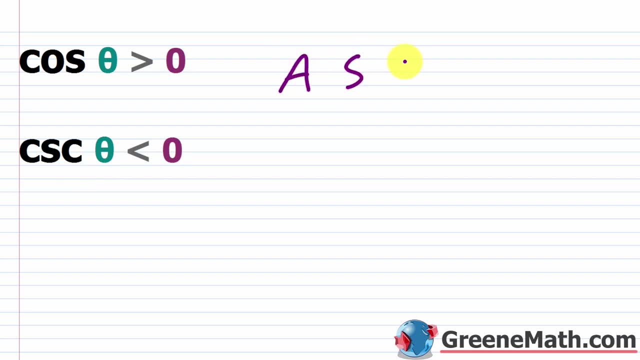 zero. Let's turn to our all students. take calculus once again: Quadrant one, quadrant two, quadrant three and quadrant four. The way I look at it is I just say: okay, well, cosine of theta is greater than zero. So where does that occur? It occurs in quadrant one and also quadrant four. 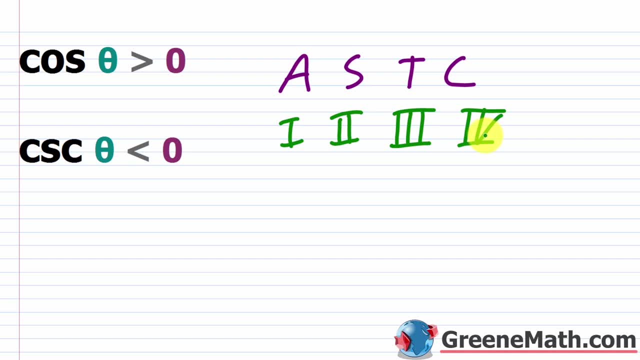 Remember, the c is for the cosine of theta And it tells you that the cosine of theta and the secant of theta are going to be positive. everything else is negative. So let me just write below this that it's quadrant one and quadrant four that satisfy that condition. Then what satisfies this condition? 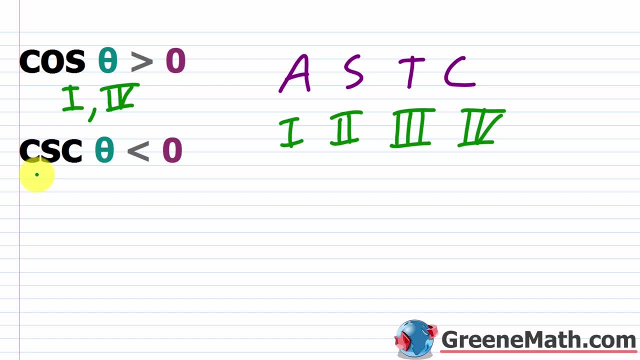 the cosecant of theta is less than zero. Remember, the cosecant of theta is going to be the reciprocal of the sine of theta. Okay, so the s stands for the sine of theta, and that's in quadrant two. So we know that in quadrant one. 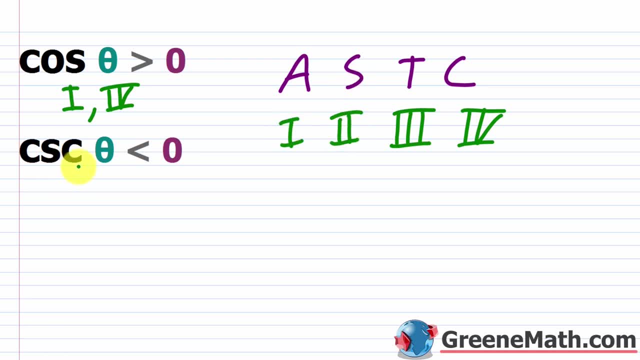 everything's positive. In quadrant two, the sine of theta and the cosecant of theta is going to be positive, And everywhere else, so in quadrant three and quadrant four, the sine of theta and cosecant of theta will be negative. So this condition is met in quadrants three and also. 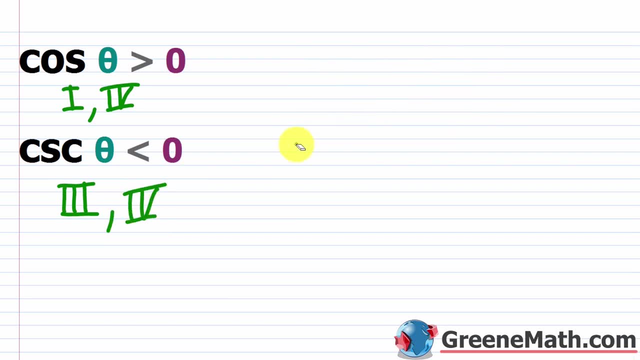 quadrant four. Let's just erase this. And now all you want to do is just say: okay, well, which quadrant satisfies both conditions? Okay, in some cases you might have more than one. In this case, we only have one: it's quadrant four. 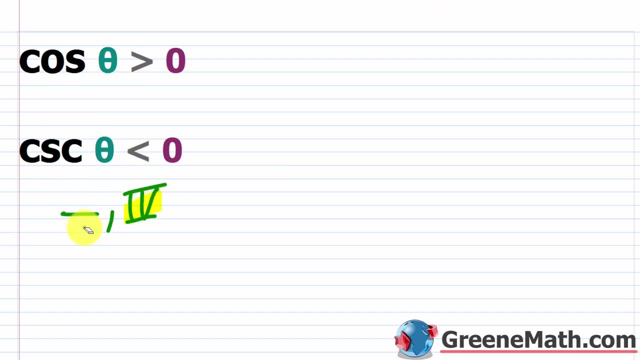 Okay. so if you wanted to answer this, you could just erase these- okay, you don't need them anymore- And you could just write out quadrant four, or a lot of teachers will just let you write the Roman numeral of the quadrant. just say quadrant four, like that for your answer. 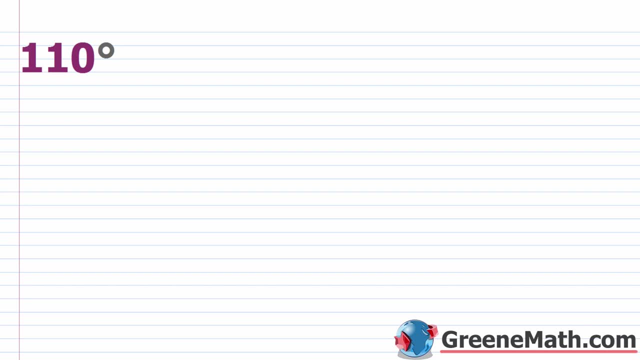 Okay, another type of example you might get is to determine the signs of the trigonometric functions of an angle When, again, it's in standard position and it has a given measure. it's 110 degrees, So this is really easy to do. This is something where you might want to make a 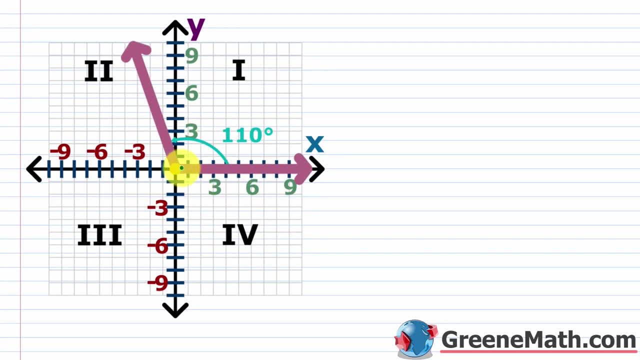 little sketch. So if this guy's in standard position again, this is going to be your initial side. here's your terminal side. we know that if it was touching your terminal side, was touching the y axis like this, it would be a right angle be 90 degrees If it goes a little further. 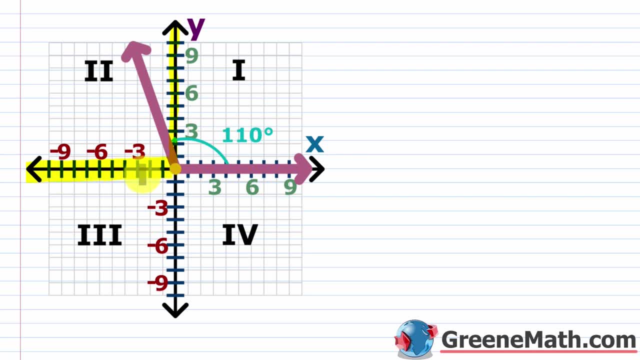 than that, but not far enough to where it's touching here, right? if it was touching the x axis, you have 180 degree angle or straight angle, So it's in between those two. So we know it will be in quadrant two, right? this would be your 110 degree angle there. 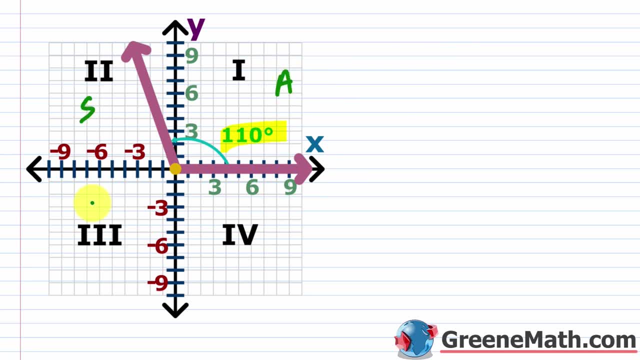 So in quadrant two, again, all students take calculus very easy. The s tells me that it's sine of theta and also the cosecant of theta. So you can say the sine of theta and the cosecant of theta. those guys are going to be positive, okay, And then the other guys are going to be. 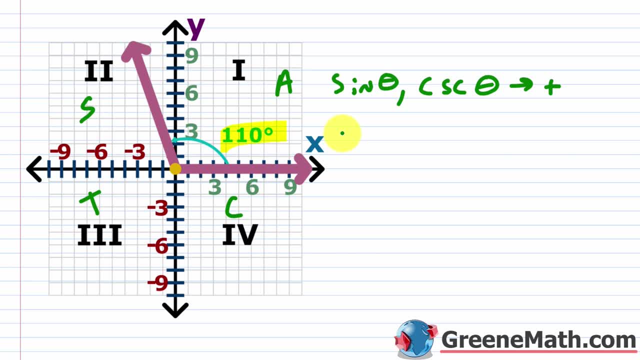 negative. So you might want to write all these out or you could say: all others are negative, depending on your teacher and what they asked for. Let's just go ahead and write them out. we'll say the cosine of theta. we'll say the secant of theta. okay, those guys are negative. 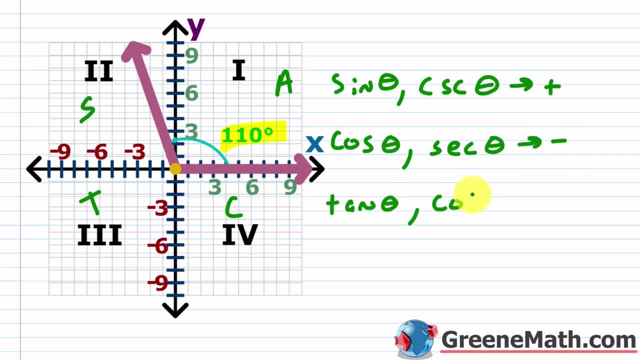 And then we have our tangent of theta and our cotangent of theta. those guys are negative as well. So only sine of theta and cosecant of theta are positive for this example. All right, another one of these. we have a negative 150 degree angle. Remember when you have a negative angle and this: 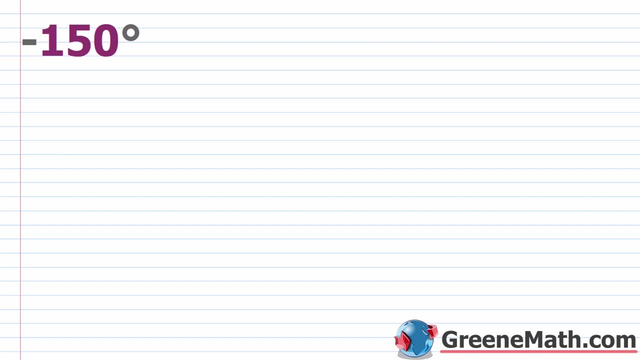 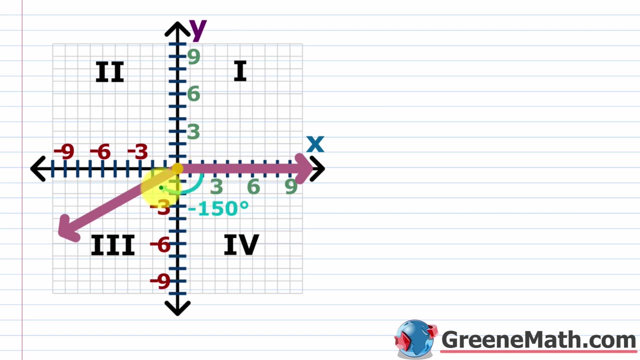 guy's in standard position. you're rotating clockwise now instead of counterclockwise. So this is negative 150 degrees and this guy's in standard position and this guy's in counterclockwise Again. you're starting here and you're rotating clockwise. So again, if you rotated this way, 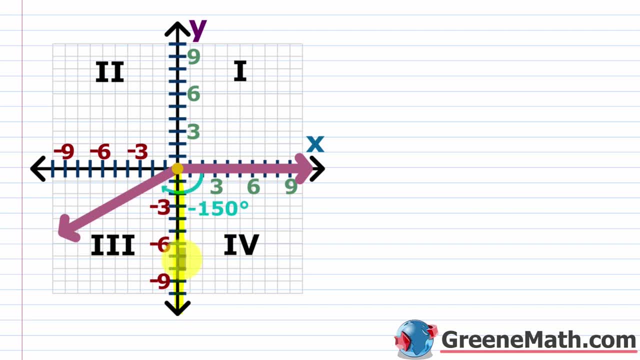 okay and you got to right here. if it's a negative angle, that would be negative 90 degrees. If it's positive, it would be positive 270 degrees. but here it's negative, So this would be negative 90 degrees, this would be negative 180 degrees. So we're between those two. again, we're going to 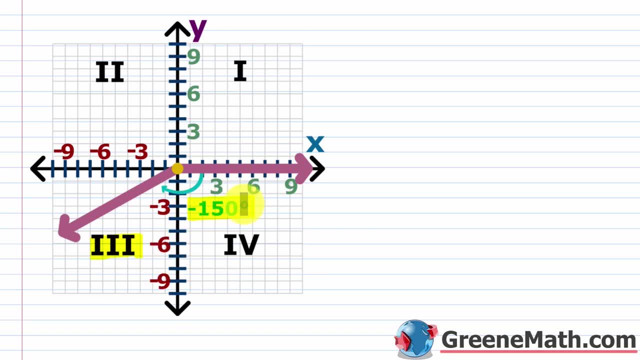 land in quadrant three here. so that's your negative 150 degree angle. So in quadrant three, just do all students take calculus. So in quadrant three you have a t for the tangent of theta and then also the cotangent of theta. those are going to be positive. Everything else will be negative. So you have your. 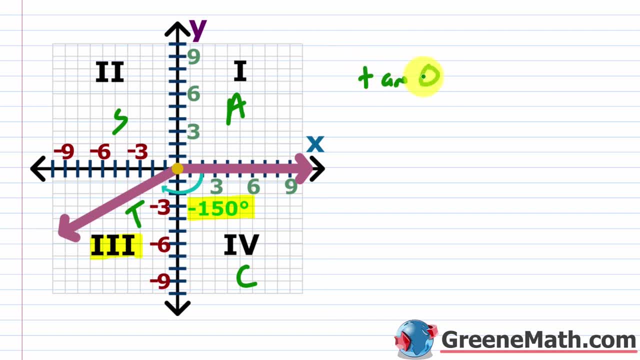 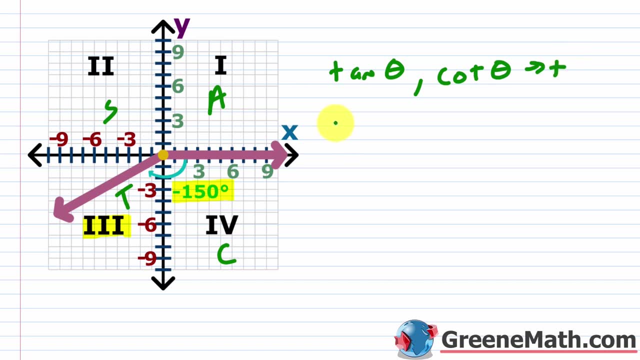 tangent, your tangent of theta, and also your cotangent, your cotangent of theta. those guys are positive and then the rest are negative. So, sine of theta and the cosecant of theta, those guys are negative, and then also your. 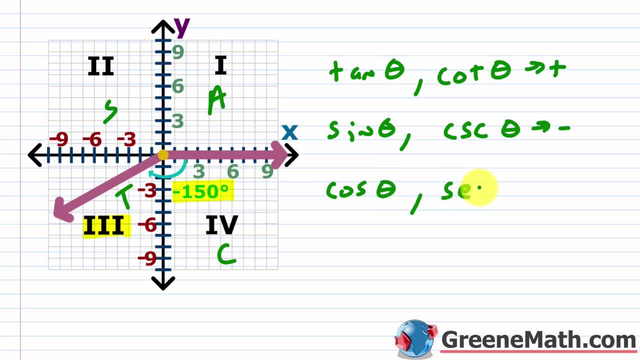 cosine of theta and also your secant of theta. okay, those guys are going to be negative as well. So, for this example, the only two that are positive are the tangent of theta and the cotangent of theta. All right, to wrap up the lesson, let's look at a very common type of problem. This is: 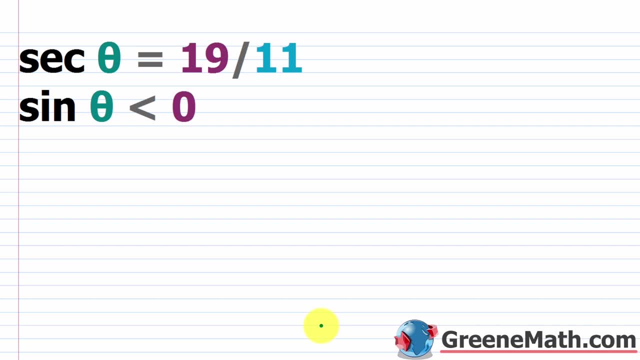 where you're given one trigonometric function value and you're either given the quadrant or you have to figure out what it is based on the information you have, and basically you want to come up with all six trigonometric function values. So here we're told. 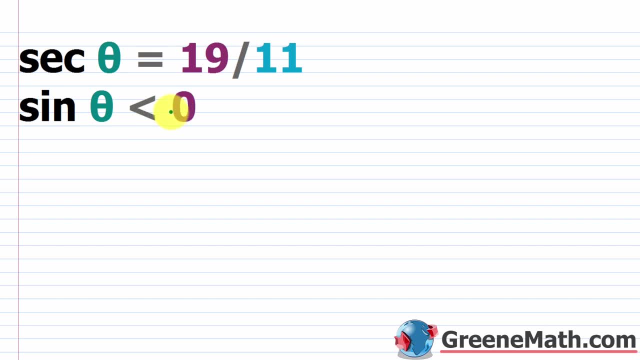 the secant of theta is 19 over 11, and the sine of theta is less than zero. So you can start this off in a few different ways and there's also multiple ways to do it. But based on what we know so far, we know that the secant of theta, we know that the secant of theta is going to be, 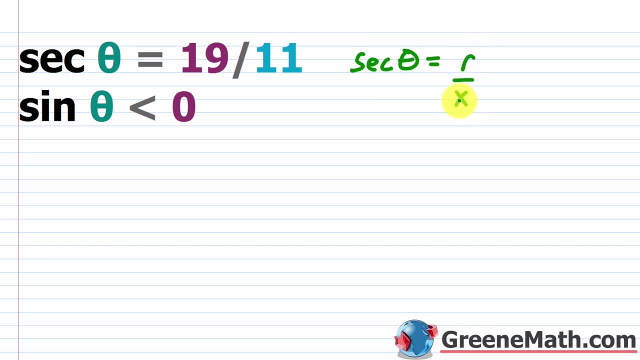 equal to my r value over my x value. Okay, so if this is 19 over eleven, I know that my r value is 19, and I that my x value is 19,. and so they come off with the tenth of two flourishing Achilles, misschien. we know this function is gonna be the second with us to take out the final. 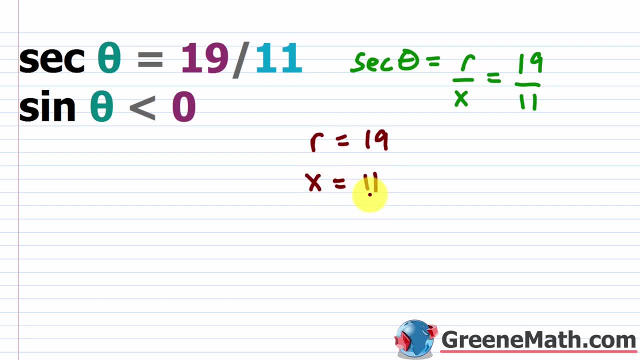 value is 11.. Okay, so that's important. So I know I'm going to need y. and how do I find y? Remember that r, by definition, is the square root of x squared plus y squared. So let's work on this really quickly. Okay, we'll come back up to this in a moment, So let's just paste this in here. so. 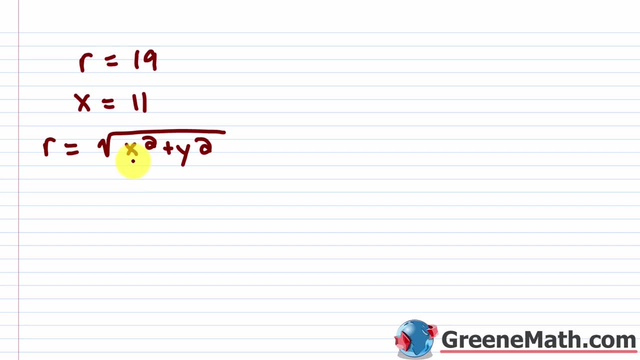 we have a lot of room to work. We know that x is 11.. 11 squared would be 121, and I know that r is 19.. So I can replace this and say that I have. 19 is equal to the square root of 121 plus y squared. 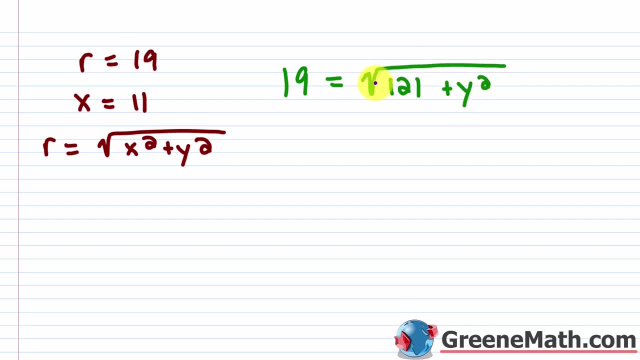 If I want to get y by itself, I first have to clear this radical. To do that, I'm going to square both sides. Squaring 19 gives me 361.. Squaring this side tells me that this would cancel with this and I'm left with the radicand, which I'm just going to change the order and say this is y. 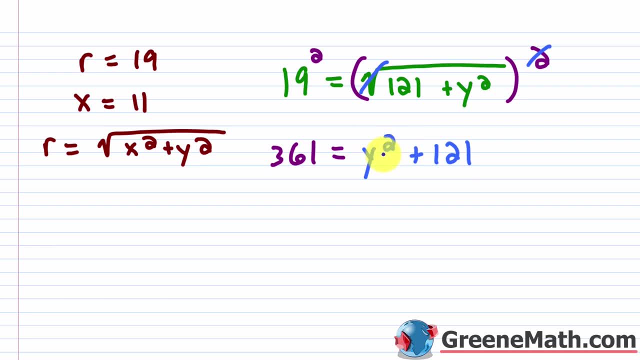 squared plus 121.. And now to isolate y, because I'm trying to solve for y. Okay, so to isolate this, I'm just going to subtract 121 away from each side of the equation. This would be 240 over here. Over here. this is gone, I'm just going to. 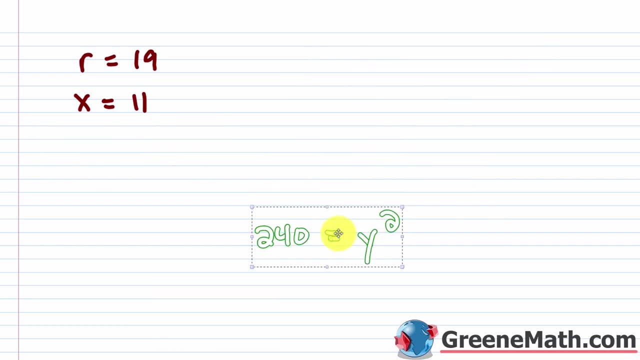 have y squared. So let me erase all of this, and I'm going to also flip the order around and put y squared on the left and 240 on the right. Again, that doesn't matter, It's just a personal preference What I'm going to do. let me just kind of scooch this down a little bit. Let's write this: 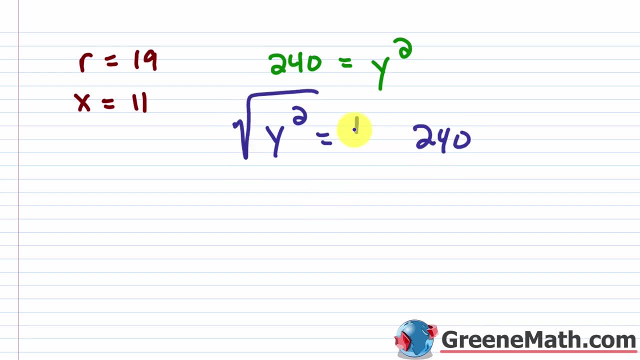 over here because we need some room. I'm going to take the square root of this side and I'm going to go plus or minus the square root This side, So 240. if you take the square root of that, you can simplify right, because 240 is 16. 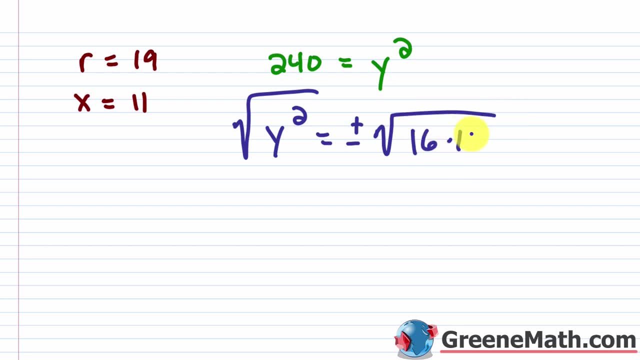 times 15.. So I could say: this is 16 times 15.. Square root of 16 is 4.. Okay, so I could just pull that out and say: this is 4 times the square root of 15.. Okay, but you do have this plus or minus out. 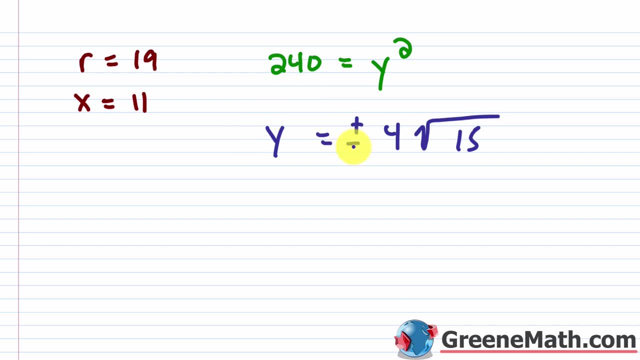 in front. that is a bit problematic here. So we need one y value. It can't be positive 4 times square root of 15 and then also negative 4 times square root of 15.. You need one or the other. Okay, so let's go back up and let's go ahead and write all the information that we know. So x is equal to. 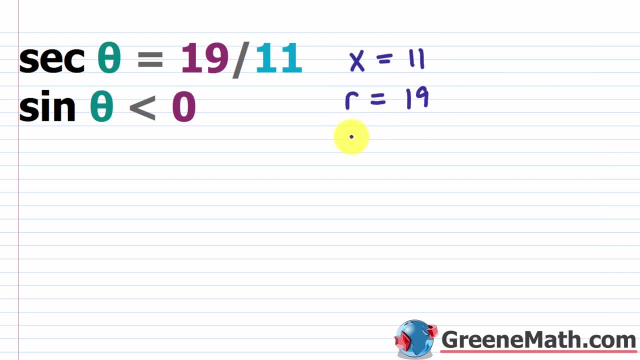 11. We know that r is equal to 19 and right now we know that y is equal to plus or minus 4 times the square root of 15.. But we need to get that down to one single value. Okay, and we're going. 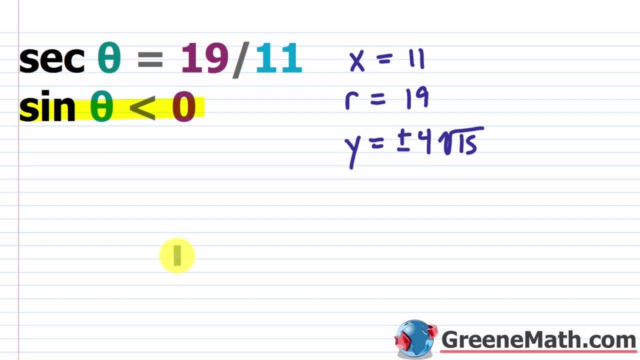 to do that with the use of this guy right here. Okay, so we're told that the sine of theta is less than zero. So where is the sine of theta less than zero? Remember, if you use your all students, all students take calculus once again. This is quadrant 1,, 2,, 3, and 4.. Okay, the s is for the sine of theta. 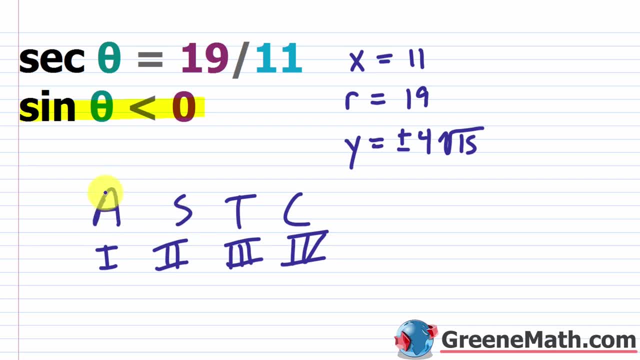 and the a is for all. Okay. so in quadrants 1 and 2 the sine of theta is positive. In quadrants 3 and 4 it's negative. Okay, so let's write 3 and 4 here. 3 and 4 here, Okay, and let's think about: 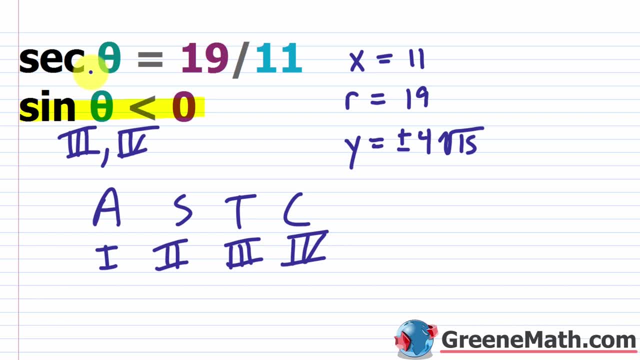 the secant of theta. Remember the secant of theta and the cosine of theta. those guys are reciprocals. Okay, the cosine of theta is going to be the sine of theta and the cosine of theta is going to be the positive, because this guy is positive in quadrants 1 and 4.. So, quadrants 1 and 4.. So again, when you 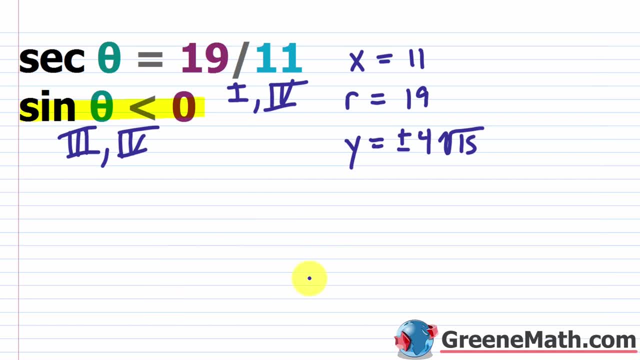 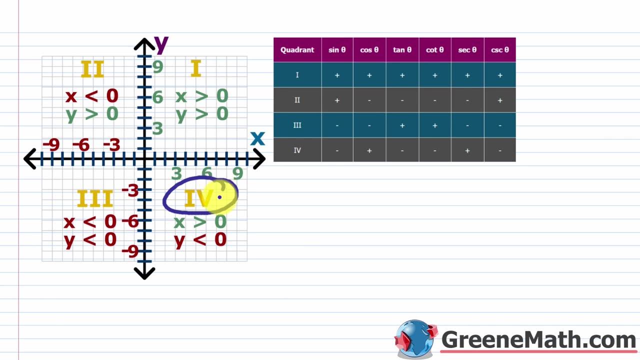 get this you're looking for. what is the quadrant that matches both? Okay, the quadrant that matches both is going to be quadrant 4.. All right, so if we know that this guy's in quadrant 4, then what are the y values in quadrant 4?? We know, if we go all the way back up here, that in quadrant 4 your y 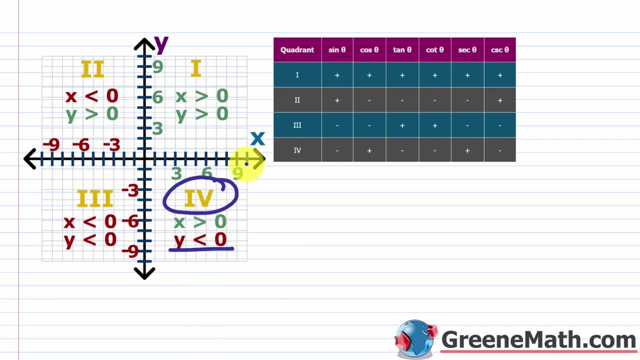 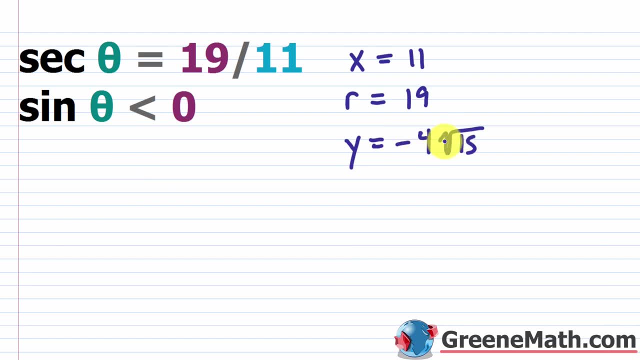 values are negative. Okay, they are negative. You are below the x-axis. So that tells me, because the y values are negative, that I don't want the positive. I want the negative 4 times the square root of 15.. Okay, so once you've figured that out, the rest of it is. 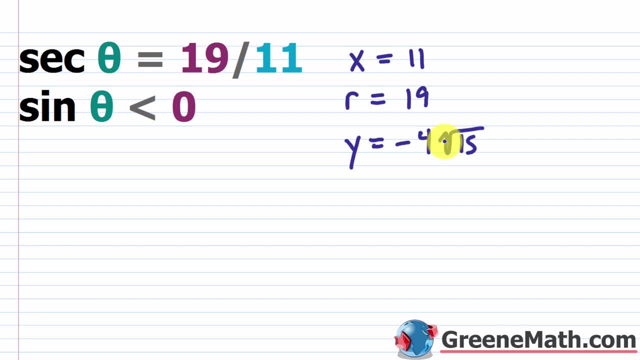 just plugging things in: Okay, knowing your ratios, having those ready, and then plugging in As we progress. we're going to go through one more lesson and we'll go through a section where we start talking about the SOH CAH TOA. Okay, we'll remember this a little bit easier, but right now we're 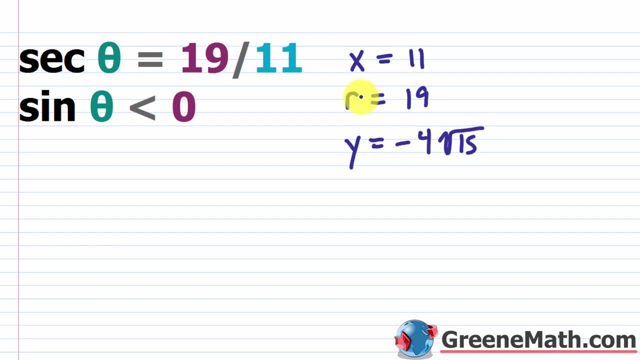 putting in in terms of x, r and y. Okay, so we have our sine of theta. Let's just start with that. That is, the y value over the r value. Then my cosecant of theta: Okay, it's the reciprocal of this. So this is the r over the y, Okay, and then let me write out the rest. So, 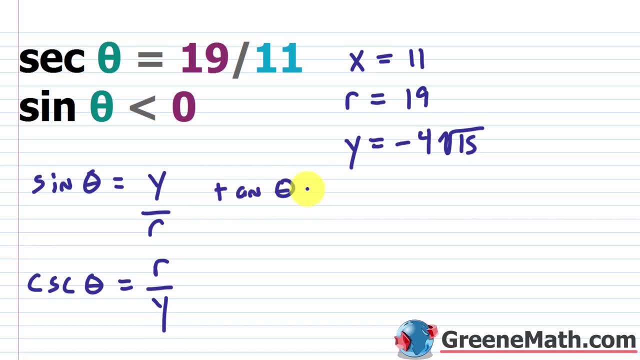 we have our tangent of theta. Our tangent of theta, This is going to be our y value over our x value, and then our cotangent of theta is going to be the reciprocal of this. So it's x over y. and then our secant of theta, Okay, is given to us, but it's r over. 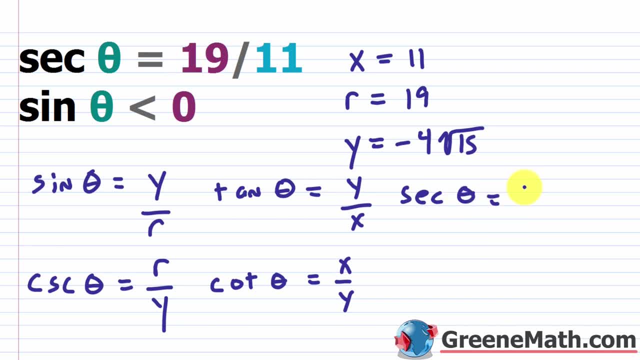 x. Okay, r over x, But in this case we already know what it is: It's 19 over 11.. Okay then our cosine of theta: Okay is x over r, But again it's the reciprocal of this guy, So we can just flip. 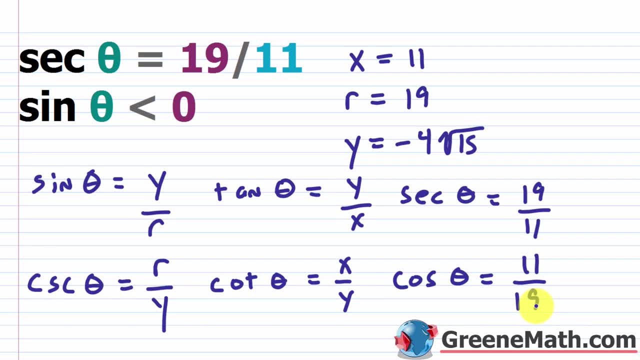 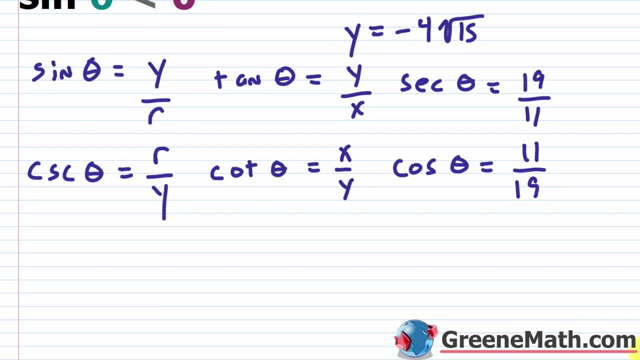 this and say it's 11 over 19.. Okay, so let's plug some things in and let's kind of get some room going here And let's see. So y, and it's a little bit off the screen here, but we'll just go back. 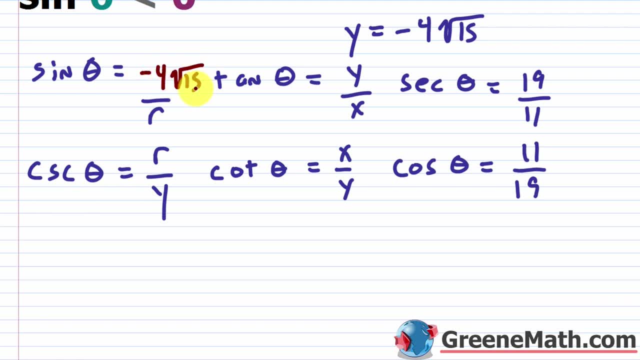 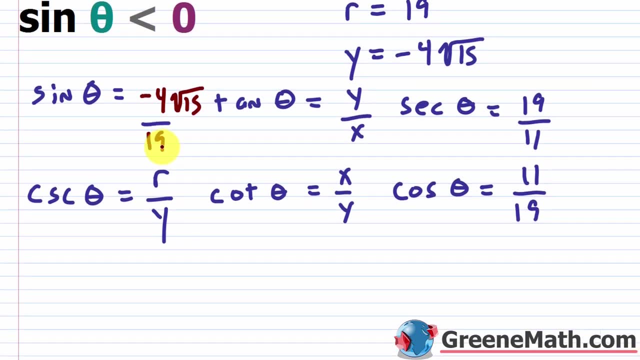 and forth. So y is negative 4 times square root of 15 and r. I know you can't see it, Let's scroll back up: It's 19.. Okay, so r is 19.. So let me just fill that in everywhere, That way we don't. 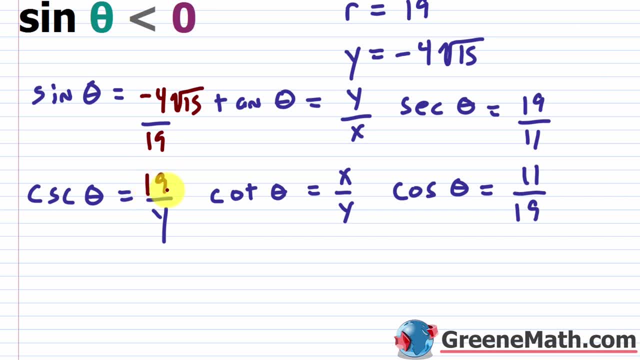 have to keep going back and forth. Okay, so those are the only two places. we need the 19.. Okay then y Let me fill that in everywhere: So this is negative 4 times square root of 15.. And let me fill that in here: Negative 4 times square root of 15.. And also here: So negative 4 times square. 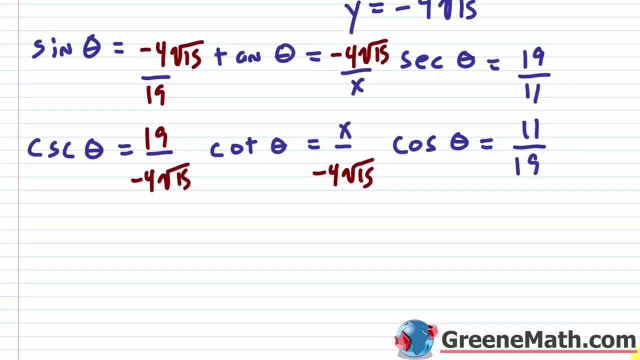 root of 15.. And x. Let's just scroll up real quick. That's going to be 11.. Okay, so we're done with that. So let's go back up here, Put 11.. And then go up here, Put 11.. For the cosecant of theta and the cotangent of theta. You need to rationalize. 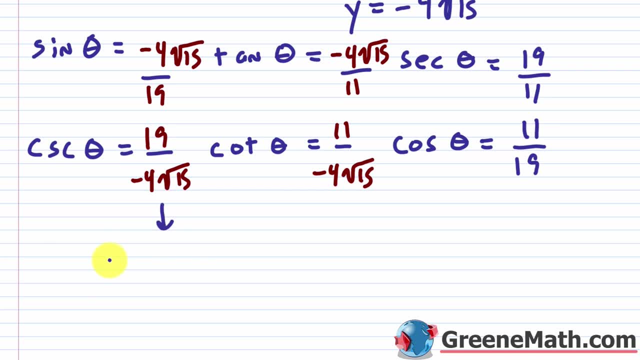 the denominator. So for the cosecant of theta, Let's just do this down here. I'll make the whole thing negative. I'll say that I have 19 over 4 times the square root of 15.. I'll multiply by the square root of 15 over the square root of 15.. Square root of 15 times square root of 15 is of: 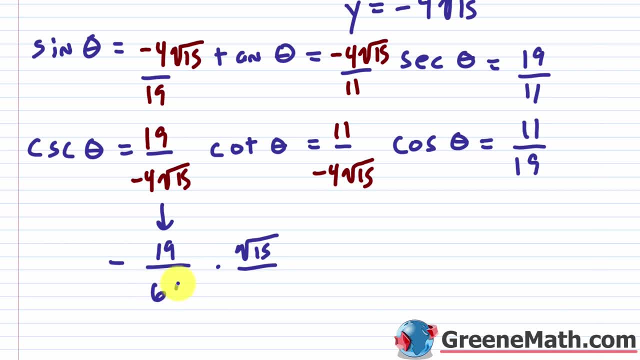 course 15.. Okay, 15 times 4 is 60.. Okay, so you really can't do anything further to simplify. So let's just erase this. Scooch this down a little bit so I have more room. I'll put the negative of: You have 19 times the square root of 15 over 60.. All right, so that one's 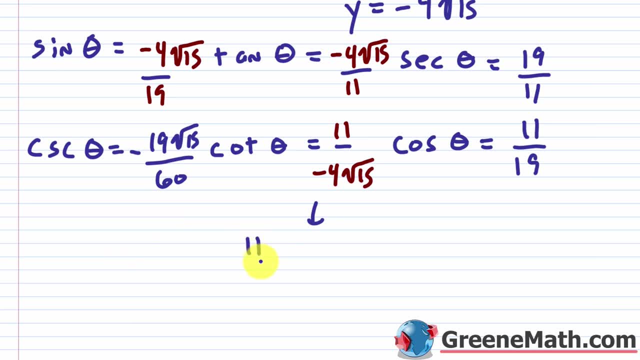 done And now I just need to rationalize this denominator. So I've got 11 over. Let's put the negative out in front. We have 4 times square root of 15.. So we'll multiply by the square root of 15. 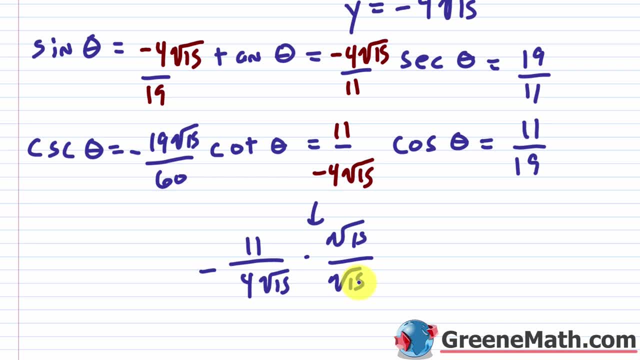 over the square root of 15 again. So we have square root of 15 times square root of 15, which is 15.. 15 times 4 is 60. So let's erase all this. Put equals, I'll make the whole thing negative. My denominator: 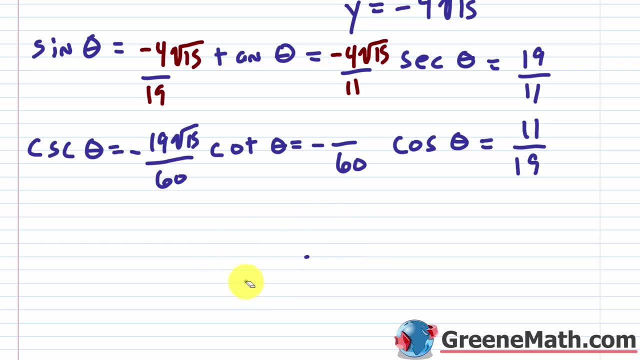 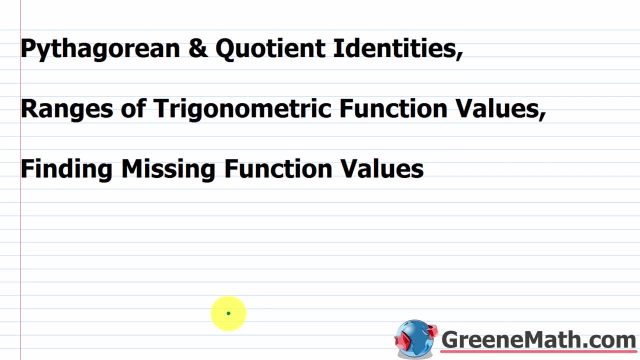 will be 60.. My numerator will just be 11 times the square root of 15.. So 11 times the square root of 15 and I'm all done. In this lesson we want to talk about the Pythagorean and quotient identities. 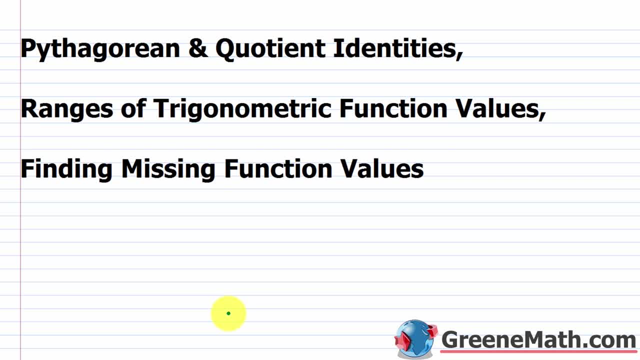 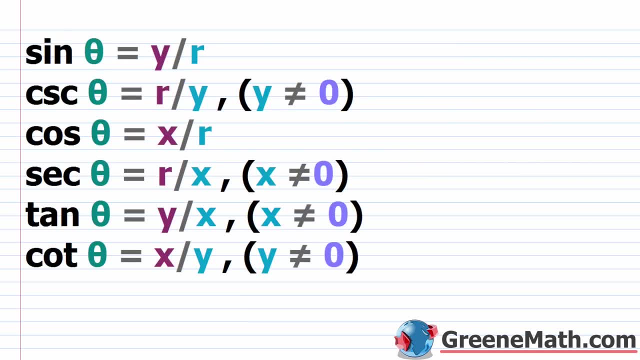 We'll look at the ranges of trigonometric function values And also we'll see some examples where we're finding missing function values. So before we jump into the lesson, for reference sake, let's go through the six trigonometric functions again. I want you guys to remember the way we've defined. 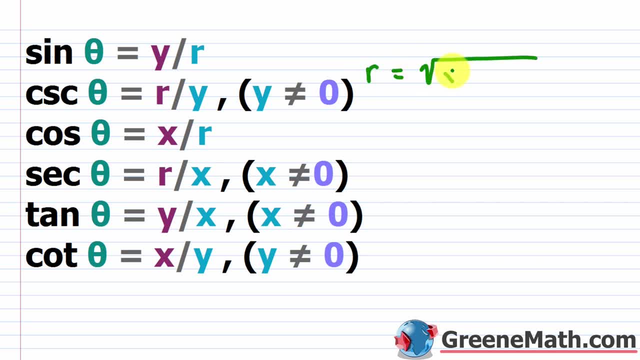 this. We've said that r Is equal to the square root of x squared plus y squared. Okay, so remember that. So I can also say, if I square both sides, that r squared is equal to x squared plus y squared. So we'll be using this. 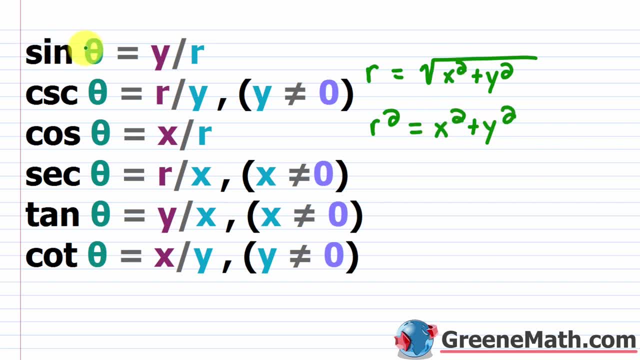 in a moment. So I want you to recall that we defined sine of theta as y over r. We defined cosecant of theta as r over y, where y is not allowed to be zero. Now you'll notice that again, sine of theta and cosecant of theta, those guys are reciprocals. Remember your reciprocal identities. 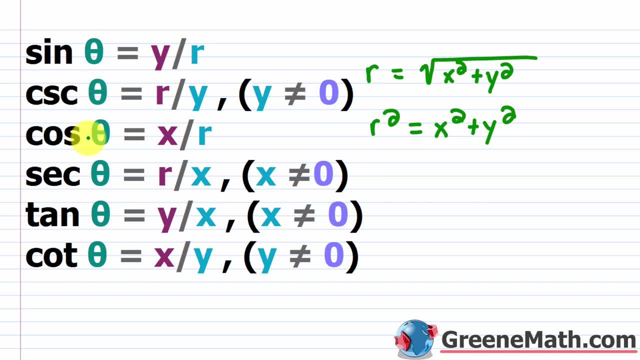 that we talked about in the last lesson. Then we have our cosine of theta which is x over r, Our secant of theta which is r over x- X is not zero. Again, these two guys are reciprocals. Then you have your tangent of theta which is y over x- X is not equal to zero- And your cotangent of theta, which 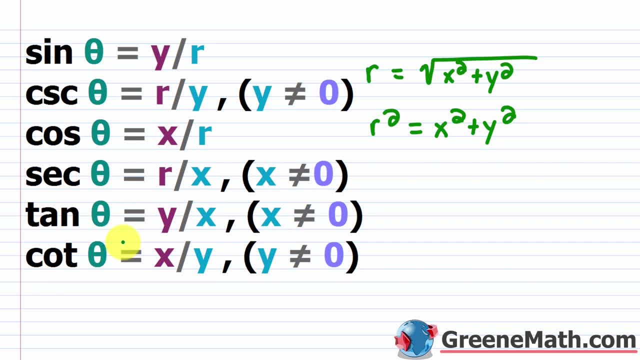 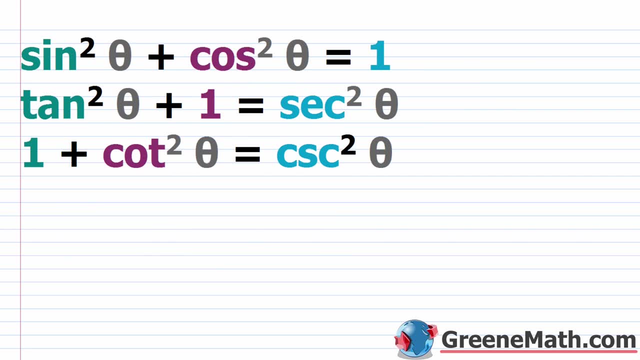 is x over y. Y is not equal to zero. Again, these guys are reciprocals. Now our first topic of today's lesson is going to be the Pythagorean identities. So you'll usually see these in your book in this exact manner. So sine squared theta plus cosine squared theta, So sine squared theta. 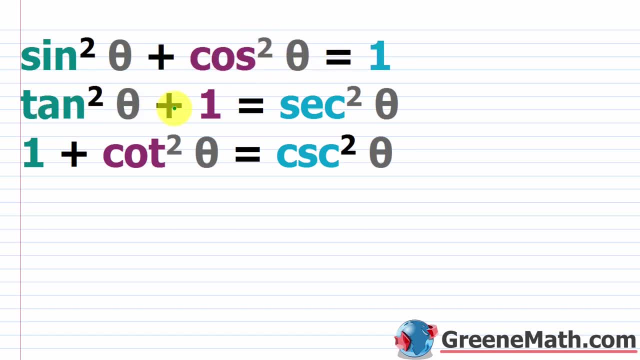 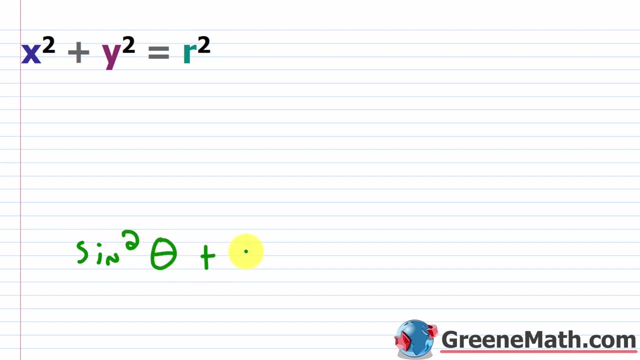 equals one. Your tangent squared theta plus one is equal to your secant squared theta. And then one plus cotangent squared theta is equal to cosecant squared theta. So how do we get the first one? So we have our sine squared theta plus our cosine squared theta is equal to one. We'll see. 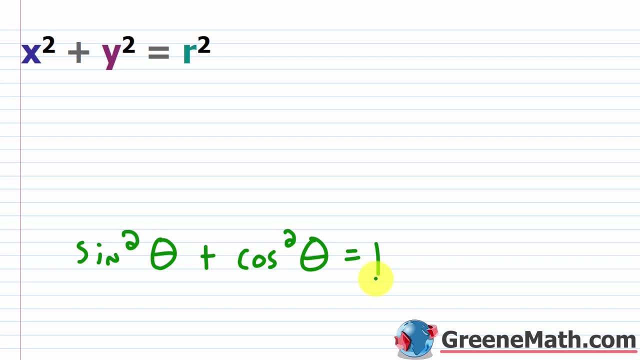 other ways to do this when we get to the unit circle. For right now we're just going to divide this by the square root of x squared, And we know that r squared divided by r squared would be one. So when we look at this guy we can say this is now going to be x squared over r squared plus y squared. 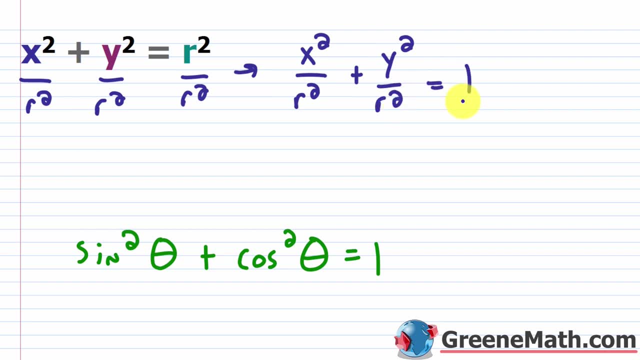 over r squared is equal to one. Okay, so now using the rules of exponents, Remember, I have a two here and a two here as an exponent, And a two here and a two here as an exponent, So I can pull that outside of a set of parentheses right, using my power rules. So I can say this is x over r, Okay. 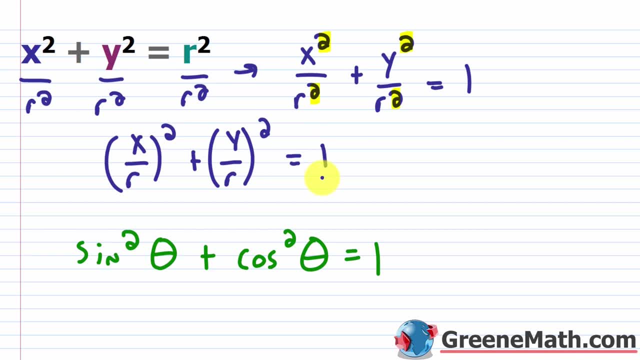 we have y over r, This guy here would be squared. This equals one. Well, by definition we just saw that x over r is cosine of theta. Okay, and then y over r is sine of theta. If we go back up again, sine of theta is y over r, Cosine of theta is x over r. So I could replace this guy right here by: 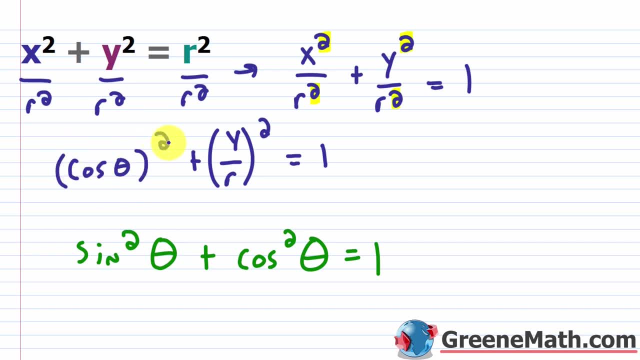 saying it's cosine of theta being squared, And I could replace this guy- Let me just kind of move this down. I could say: this is sine of theta being squared and this equals one. Okay, so I could apply my exponents and use the commutative property to get into this form here I can write this as: 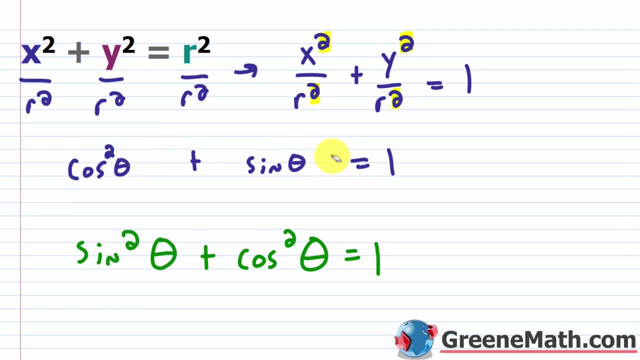 cosine squared theta- Okay, and I could write this as sine squared theta- Okay, and then I could just switch the order, because, again, this is just addition. So when you add two things together, the order doesn't matter. So that's how we get to this form right here. So let's look at the other. 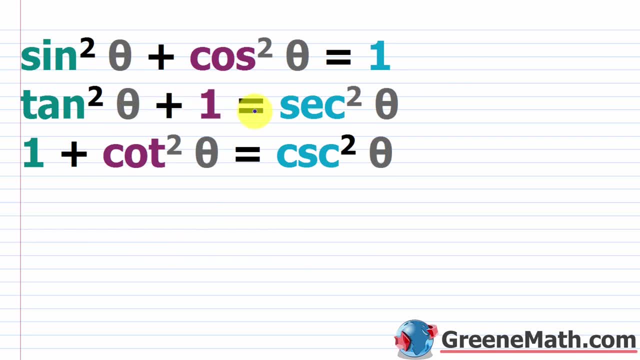 ones. So we have tangent squared theta. plus one is equal to secant squared theta. So to get this, let me just erase everything. You're just going to divide everything by x squared. now, Okay, quite easy. So divide this by x squared, This by x squared, This by x squared, And we know that this guy is. 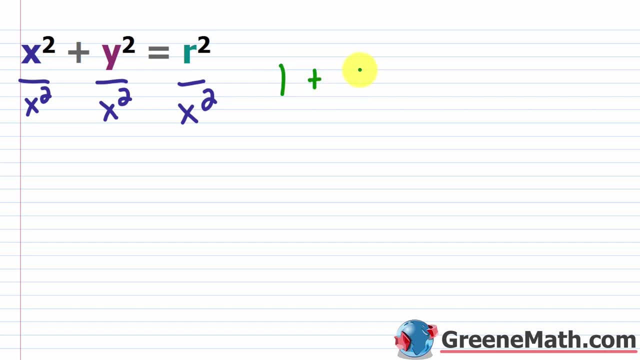 going to be one. All right, so we know we would have one plus You'd have your y, And I'm just going to write this as y over x. this guy squared- Because we know we do that step anyway- Is equal to r over x. this guy squared, What is y over x? We know that this is the tangent of theta. 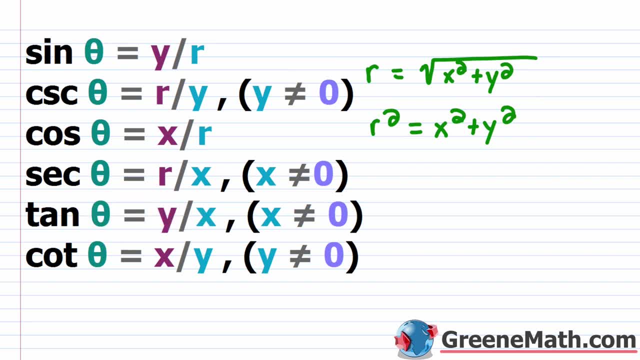 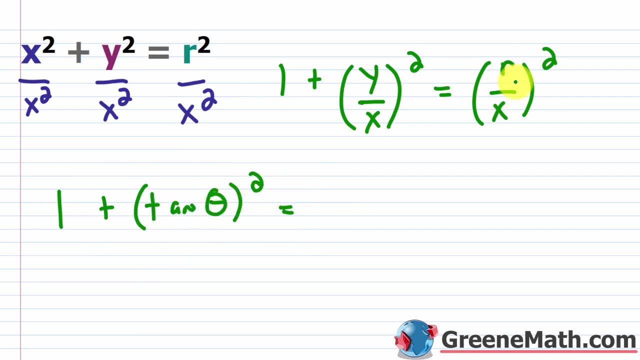 So we go back up Again. y over x is the tangent of theta, So you can replace that. You can say: this guy squared is equal to what is r over x. Well, r over x is the secant of theta. Okay, so we go. 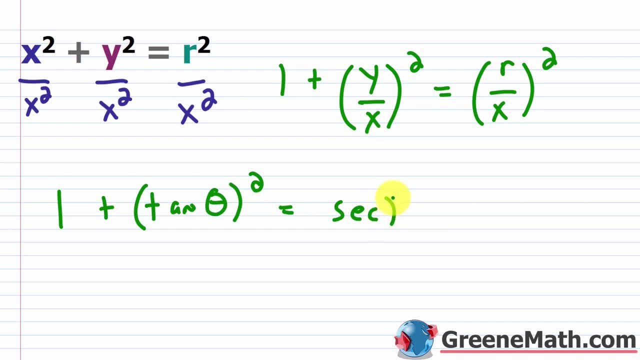 back and we say: this is the secant of theta- Let me make that a little bit better- The secant of theta, This guy is being squared. And again you can apply your exponents and just say: this is the tangent squared theta, Okay, and this is the secant squared theta, Okay. and then the way we 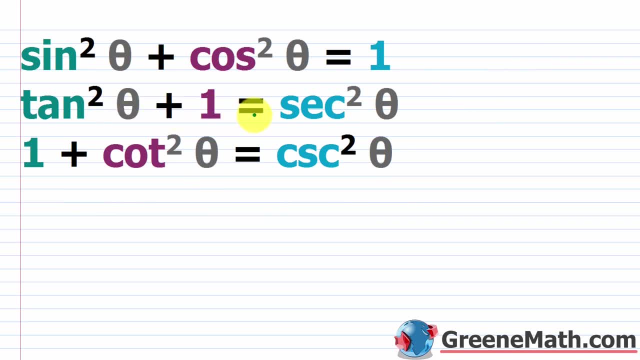 had, it was tangent squared theta plus one is equal to secant squared theta, So all we'd have to do is just rearrange this. So we're going to do this, We're going to do this, We're going to do this. 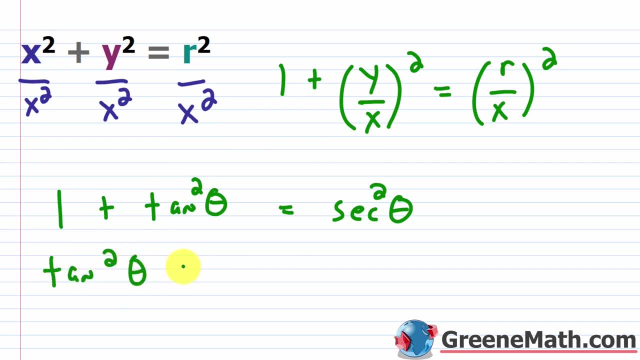 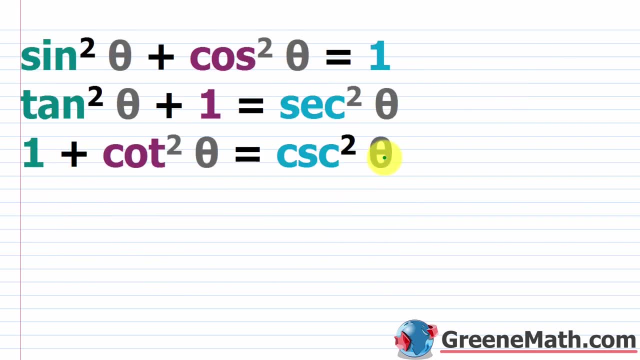 And say: okay, I have the tangent squared theta plus one equals secant squared theta. Let's look at the last one, Which is this guy right here. So one plus cotangent squared theta equals cosecant squared theta, And to get this one I'm just going to divide everything by y squared And again it's. 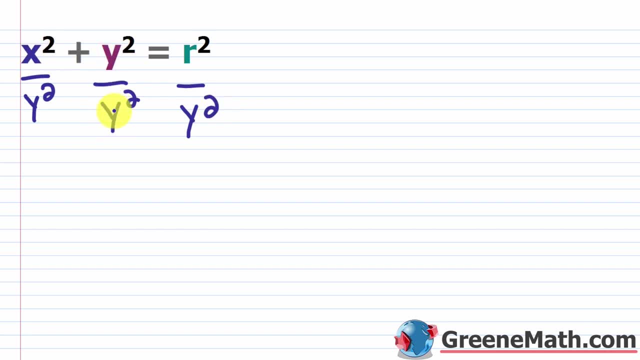 going to be the same trick overall. So now this guy is going to be one. So I would write this as: x over y. This guy would be squared. Plus this would be one. Plus this equals You'd have r over y. This guy is squared. Okay, So x over y. We know that's. 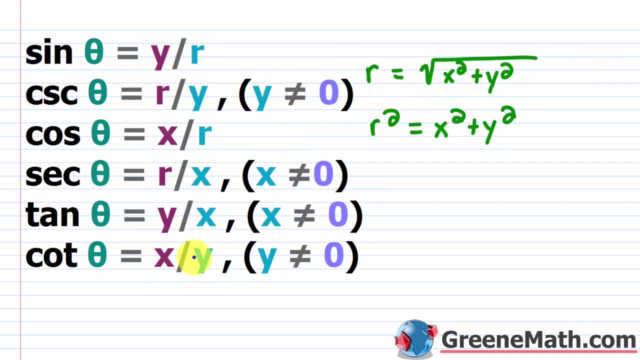 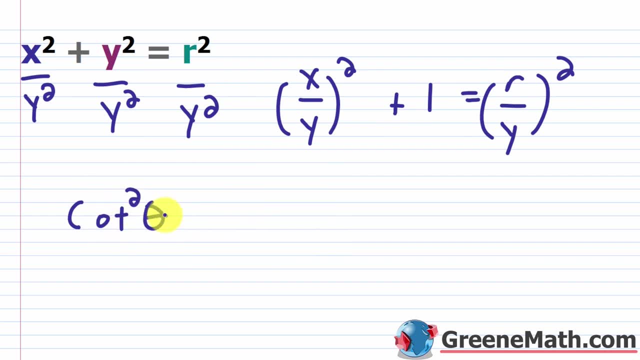 cotangent Right. So cotangent of theta, X over y is the cotangent of theta. So let's go ahead and say we have cotangent of theta And I'm just going to put cotangent squared of theta. We know it would. 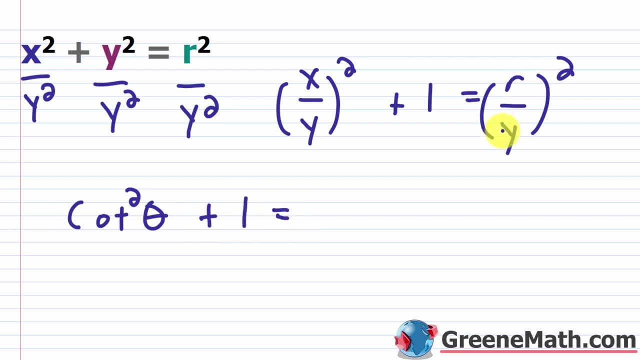 end up being that anyway. So then plus one equals What's r over y. So r over y is cosecant of theta, Okay. So I'm going to say this is cosecant squared of theta, Okay. And again, if I go, 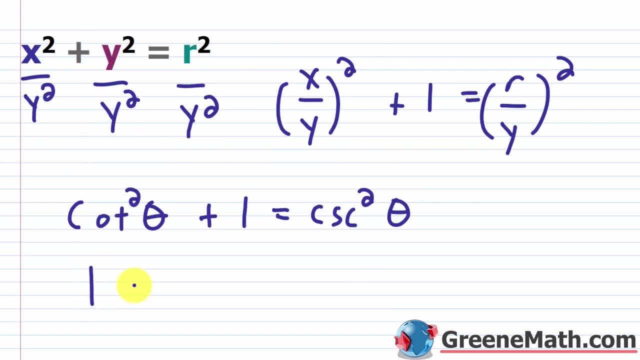 back. all I have to do is switch the order of these two, So I'll just write this as one plus cotangent squared theta is equal to cosecant squared theta. Okay, So that's where those three guys come from. Not very difficult to derive overall, But it's something you might. 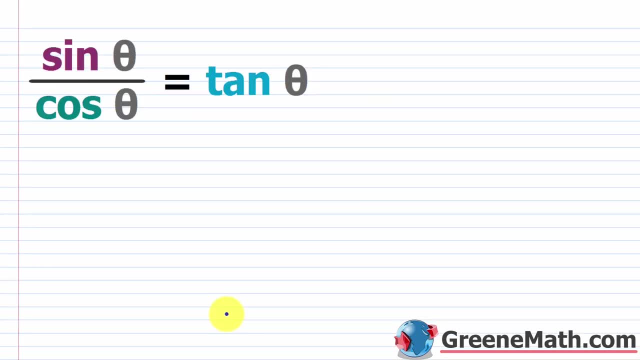 see in your book and get a bit confused about. All right. So now let's move on and look at the quotient identities. These are a lot easier to understand. You have sine of theta over. cosine of theta gives you the tangent of theta. Remember, sine of theta is y over r. 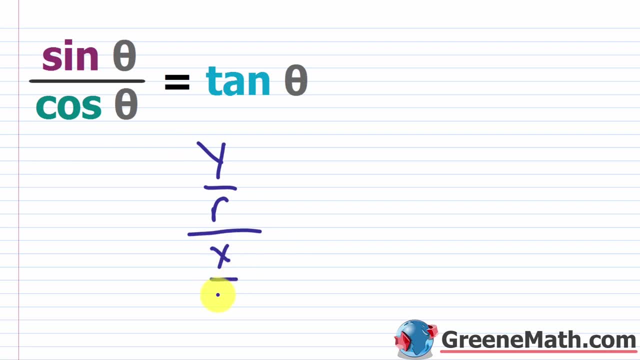 Cosine of theta. if I divide it by that, it's x over r. Well, what do we do here? This is y over r times the reciprocal of this, which is r over x. Okay, So the r's cancel and you get y over x. 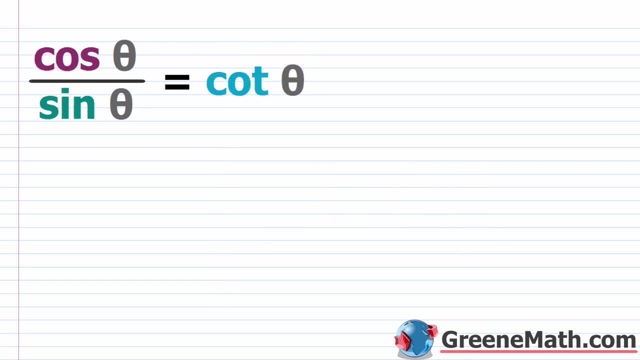 which, by definition, is the tangent of theta. So the other one is the cosine of theta over the sine of theta gives you the cotangent of theta. Well, before you even do this, remember the tangent of theta, Okay, Which is y over x, and the cotangent of theta, which is x over y. Those guys are. 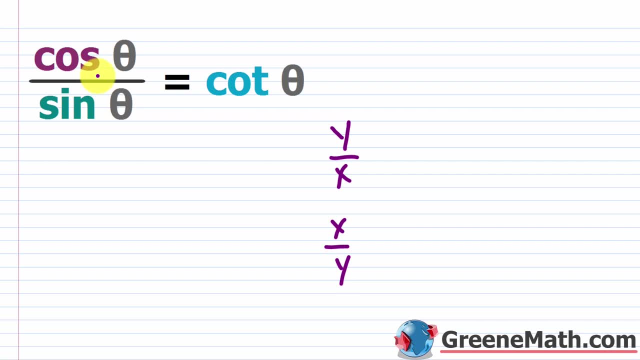 reciprocals. Well, look at what I did here. I just took the reciprocal of just what I was working with. I had sine of theta over cosine of theta. Now I'll flip that. I have cosine of theta over sine of theta. So of course I'm going to get the reciprocal of what I got before, which is the 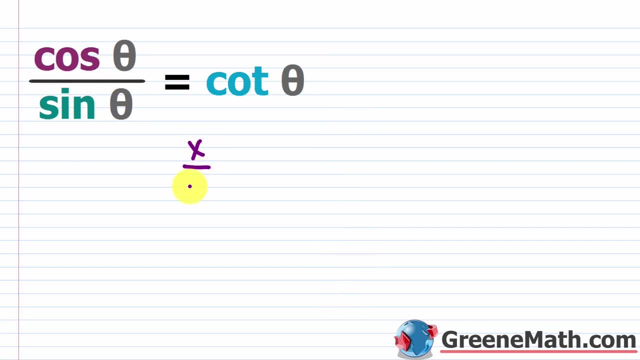 cotangent of theta. Okay, So now all I would have is x over r, divided by y over r. This is x over r times the reciprocal of this, which is r over y. Okay, So these cancel and you get x over y, which? 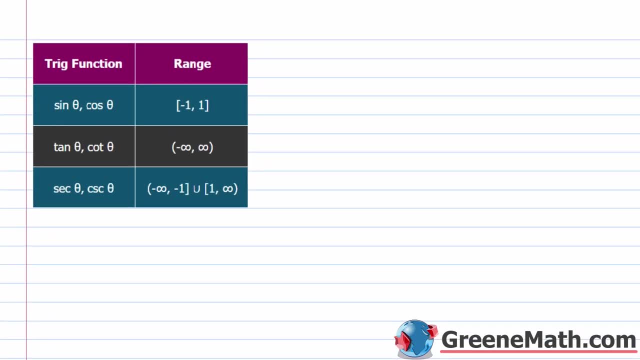 again, is the cotangent of theta. Last thing before we start doing these problems: In a lot of cases you need to know the ranges of the six trigonometric functions, because you'll go to solve a problem and you might get something that's not possible, but you think that it is possible and we'll see that on the first example. 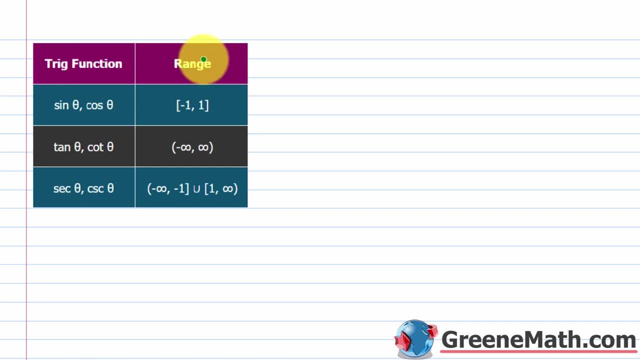 I'll show you exactly what I mean. So when you look at your trig functions, you have this range. when you think about sine of theta and cosine of theta, the value needs to be from negative one to one, including negative one and one, but in that range, Okay. When you work with tangent of theta, 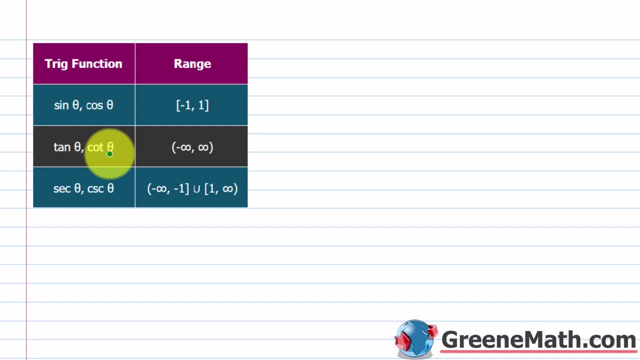 it can be any real number. Okay, It can be any real number When you work with the secant of theta or the cosecant of theta, well then you can really say: this is just that the absolute value has to be one or larger. Right, Because you can have from negative infinity up to and including negative one. 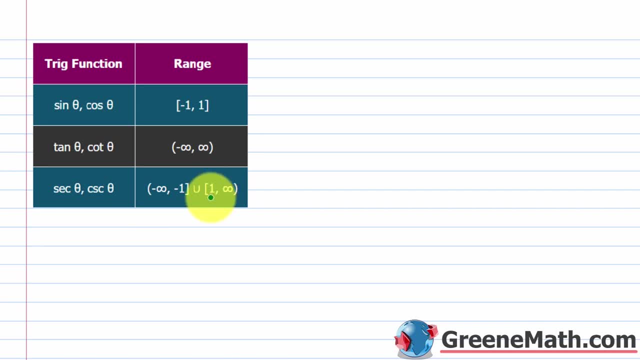 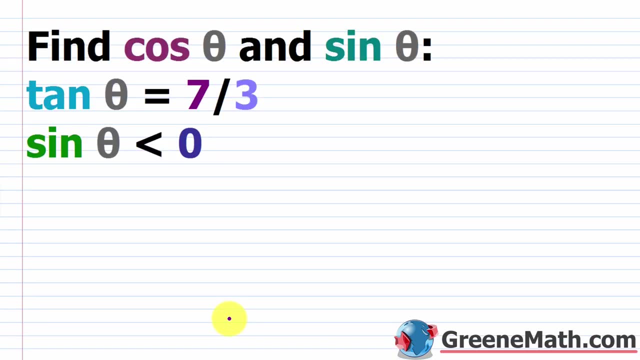 and then also from one out to positive infinity. Okay, So basically, the absolute value needs to be one or larger. Okay, It can't be less than that, All right. So let's look at our first example. here We're going to use the identities to find cosine of theta. 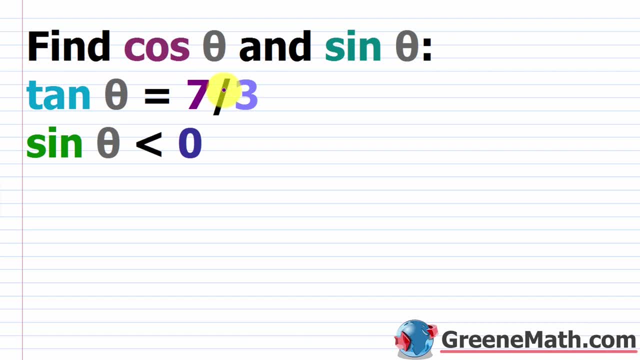 And sine of theta, given the fact that the tangent of theta is seven thirds and the sine of theta is less than zero, meaning it's negative. So, first and foremost, think about the quadrant you're going to be in. Remember that all students take calculus. So we have our four. 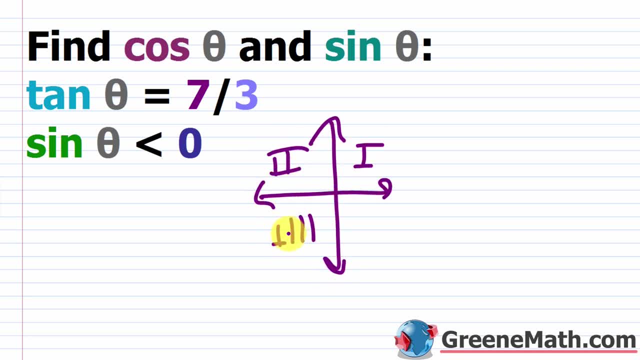 quadrants One, two, three. I'll put four marks. there should be three, So three and then four. Okay, So all students take calculus, All right. We know that t stands for the tangent of theta And also the cotangent of theta, the reciprocal. So it's positive in quadrants three and also in. 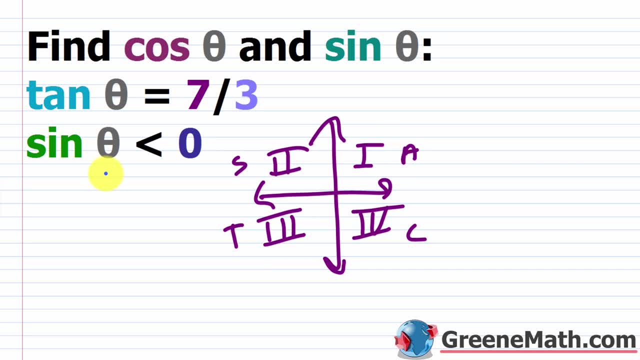 quadrant one because everything's positive in quadrant one. Sine of theta is negative. Okay, In quadrants three and four, because the s stands for the sine of theta. So we know that we're in quadrant three because it meets both criteria. Right, It's going to be positive for the tangent. 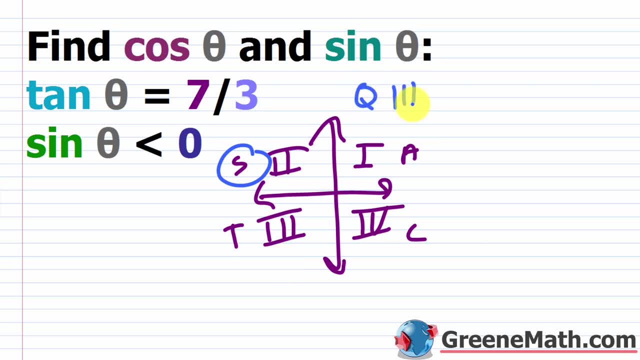 of theta and negative for the sine of theta. So we will be in quadrant three. Okay, So keep that in mind when you get stuff to know whether it's positive or negative. Now the other thing is- and this is a very common mistake, Remember, we just said that the tangent of theta is equal to. 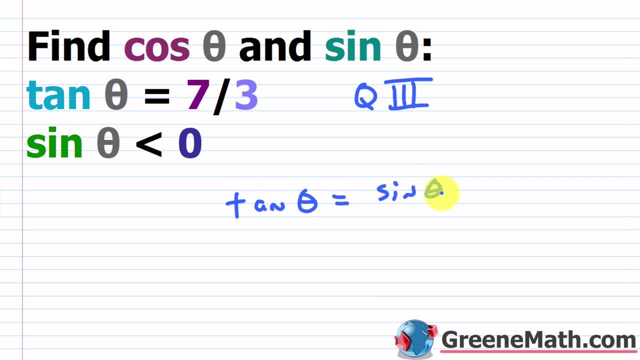 the sine of theta, the sine of theta over the cosine of theta. So what students do is they say, okay, well, sine is negative And I know that tangent is positive. So what they'll do is say, okay, well, this is going to be negative. seven over negative three. Okay Over negative three. 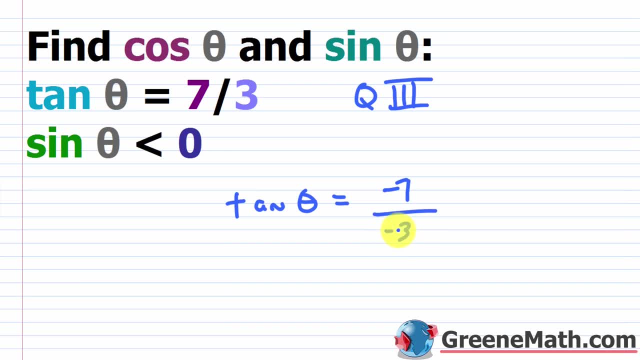 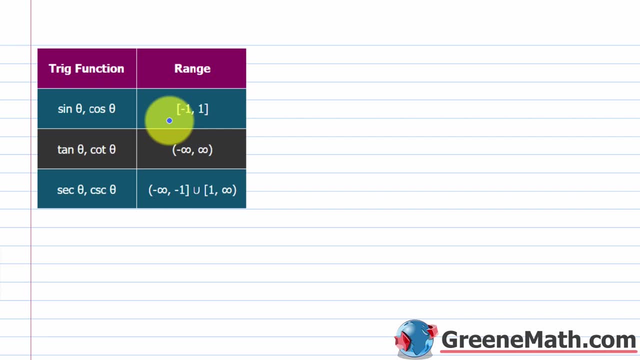 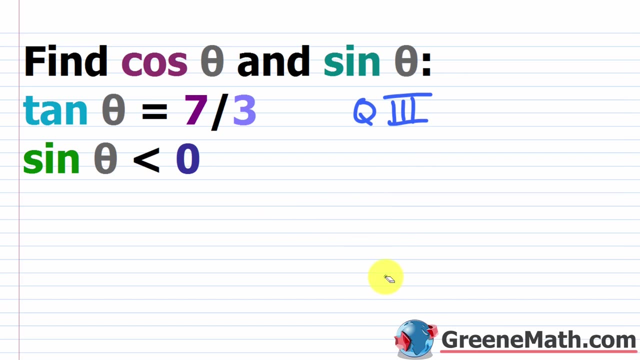 And they think they're done with the problem. This is a very common mistake. Why doesn't it work out this way? Remember, the range for sine of theta is negative. So what we're going to do is we're going to take our Pythagorean identity that includes the tangent of theta, and we're just. 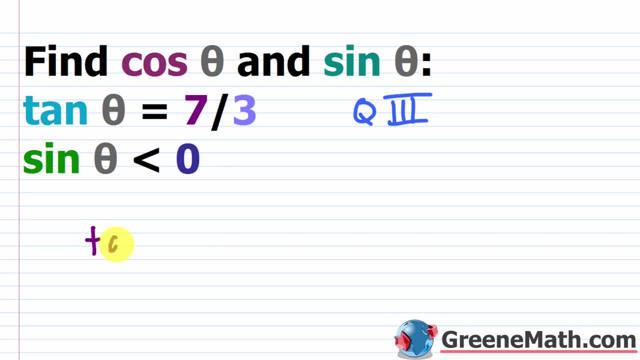 going to plug into that. So we have the tangent squared of theta, Okay, Plus one equals the secant squared of theta, Okay. So you might be saying, why would we plug into that? Well, we're trying to find cosine of theta and sine of theta. Remember, the secant of theta is the. 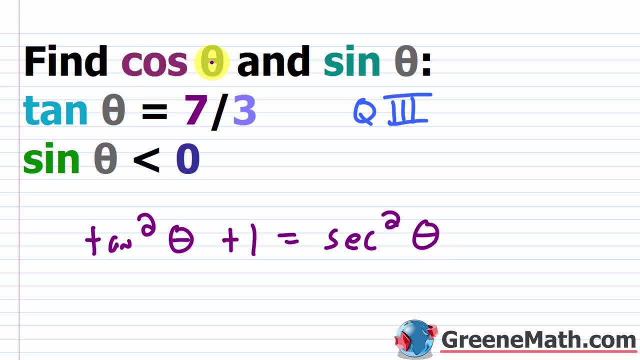 reciprocal of the cosine of theta. Okay. So if we find the secant of theta we can flip it. We'll have cosine of theta, Okay. And once we've done that, we know that our other identity involves sine of theta and cosine of theta. We can plug into that and figure out our sine of theta. 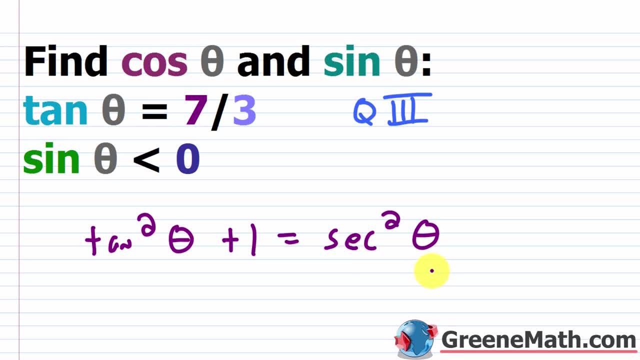 So let's just go ahead and knock this out. We're given that the tangent of theta is seven thirds, So you would want to plug in here. Okay, Remember this guy's being squared. So when you plug in here, make sure that you square this. 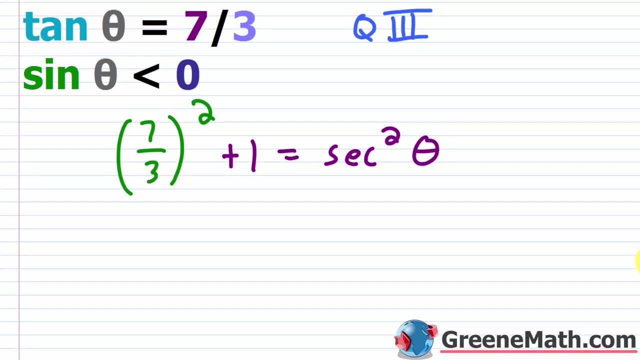 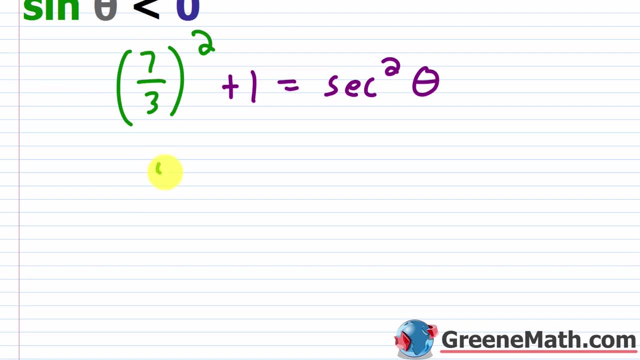 guy. It's very important. Okay, So we come down here Once you've plugged in. the rest of this is really really easy. You're just doing some basic algebra. Seven squared is 49.. Three squared is nine. Then you're going to add one to that, So get a common denominator. Let's just say this is: 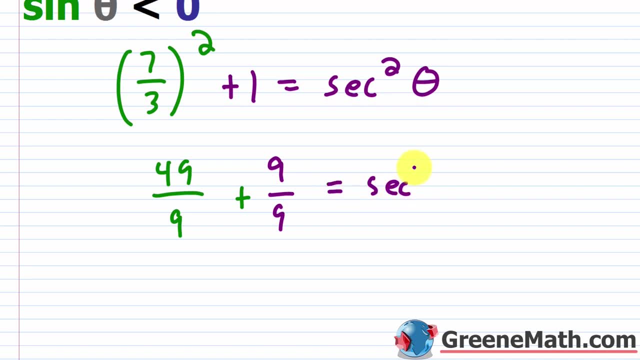 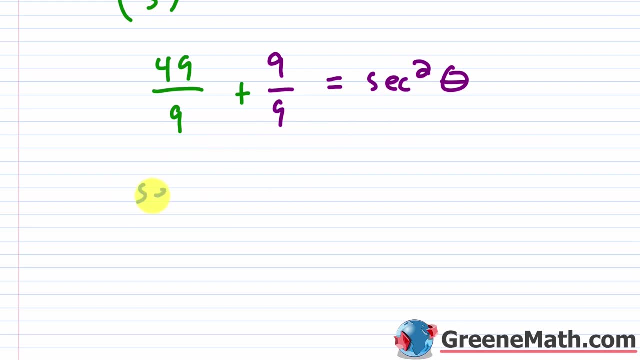 nine over nine. Okay, This is equal to secant squared of theta. Okay. So let's go down a little bit more. I'm going to flip this around and put this guy on the left. So secant squared of theta is equal to: 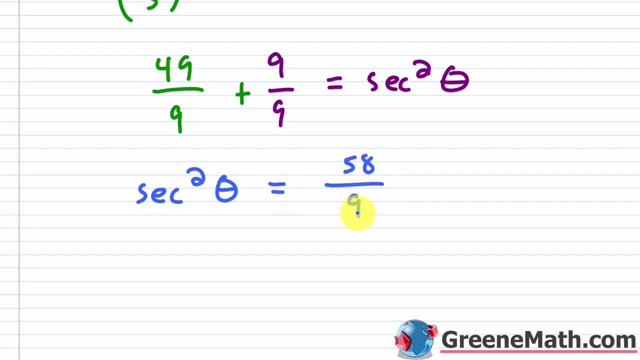 49 plus nine is going to give me 58. And this is over nine. Now to get this in the form of secant of theta. Okay, What I want to do, since this is being squared, I want to take the square root of. 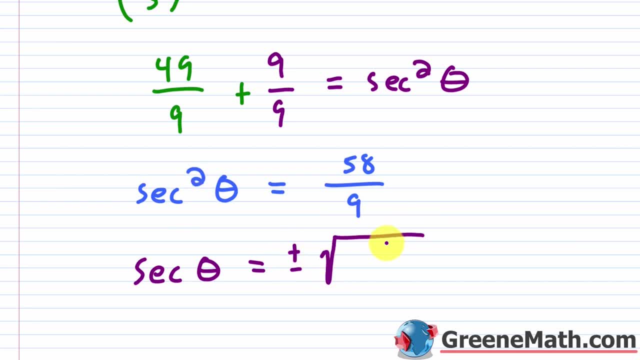 each side. Remember, on this side I want to go plus or minus. Okay, The square root of 58 over nine. I'm only going to need one of these. Remember, I'm in quadrant three. That's what we did that to. 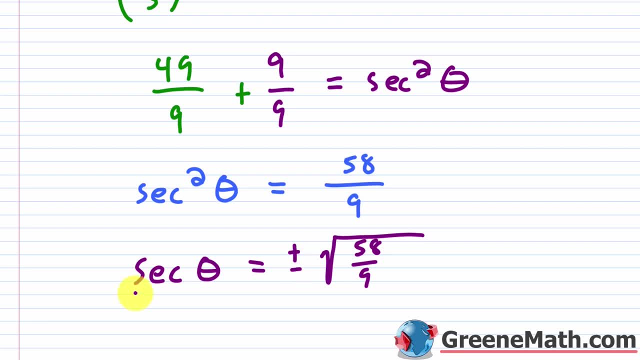 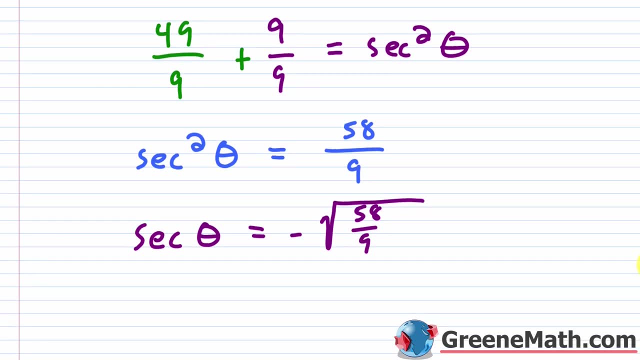 begin with, I'm in quadrant three. In quadrant three, the secant of theta is going to be negative. So throw out the positive one, You just need the negative. Okay, That's all you want. So let's scroll down a little bit and we'll say the secant. 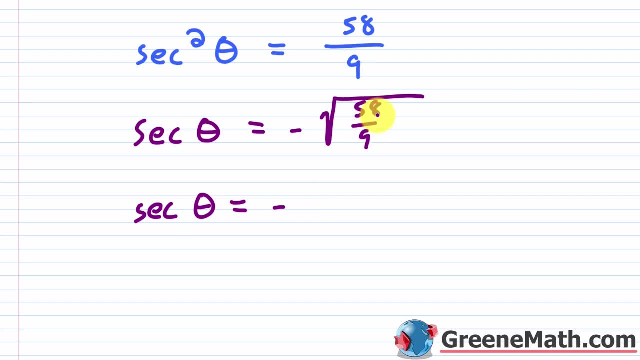 of theta. Okay, It's going to be equal to the negative of. this would simplify, because the square root of nine is three, So I'll say the square root of 58 over three. Okay, So we're not looking for the secant of theta. Of course we want the cosine of theta And I know this is a bit. 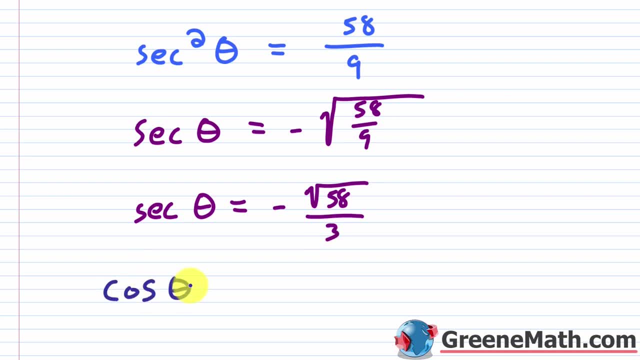 tedious, but the cosine of theta is found by flipping this guy, So this is equal to the negative of three over the square root of 58.. Now, when you have an answer with the square root in the denominator, you typically want to rationalize the denominator. So let's multiply this by the. 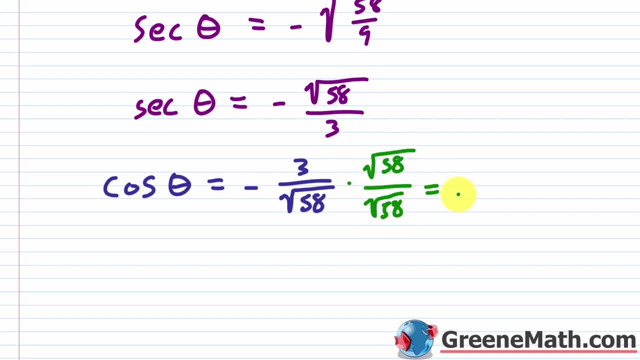 square root of 58 over the square root of 58. And that would give me an answer of the negative of three times the square root of 58 over 58.. Okay So, that's my cosine of theta. I also want to define sine of theta. Okay So, sine of theta. what does that equal? to Remember sine squared. 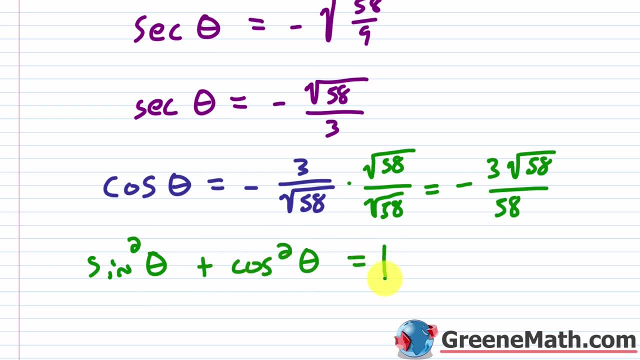 theta plus cosine squared theta is equal to one. Well, I can plug in for the cosine squared theta. I'm just going to plug in the non-rationalized version here. So I'm going to put negative three over square root of 58.. Okay, You don't need the rationalized one, because this is. 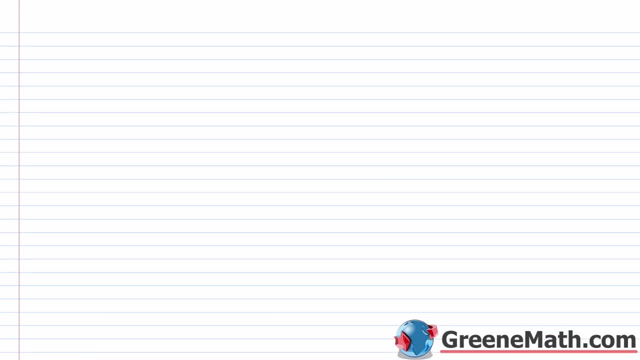 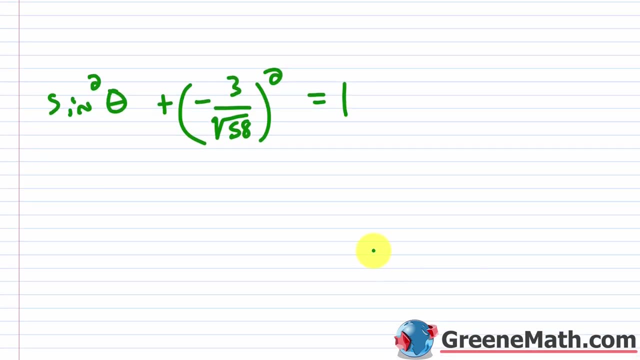 not the final answer. Let's copy this because we're going to run out of rum. go to a fresh sheet here and let me erase this- We don't need that- and scroll down a little bit more. So if I square this, let's just go ahead and put sine squared. 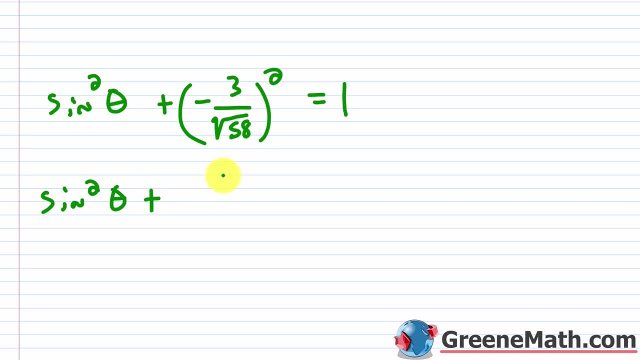 theta plus by square this, I'm going to get positive, of course, nine over 58 and this equals one. Okay, So all I got to do is subtract this away from each side of the equation, So I'll have sine squared. theta is equal to one minus nine over 58. And, of course, we just get a common. 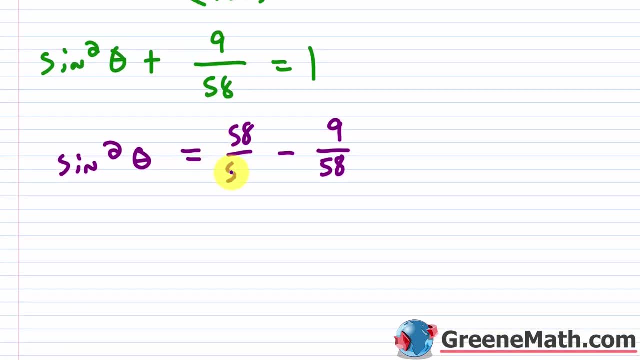 denominator going. So I'm going to say: this is 58 over 58, and 58 minus nine would be 49. So this is 49 over 58.. So this is 49.. Okay, So to get sine of theta, remember, you're taking the square root of each side, So do you? 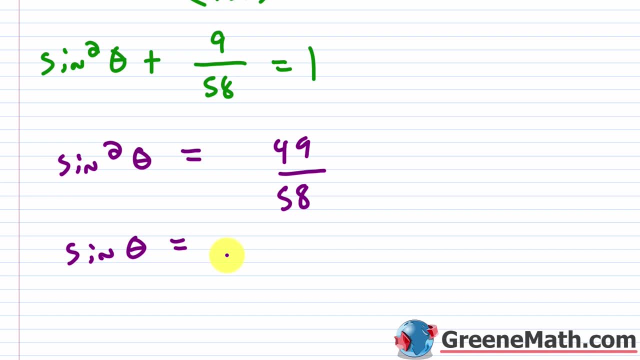 want the positive or the negative square root. Remember, sine of theta is going to be negative in quadrants three and four. We're in quadrant three, So it's going to be negative. So I want the negative square root of 49 over 58.. Okay, Let me make that reach all the way. And, of course, 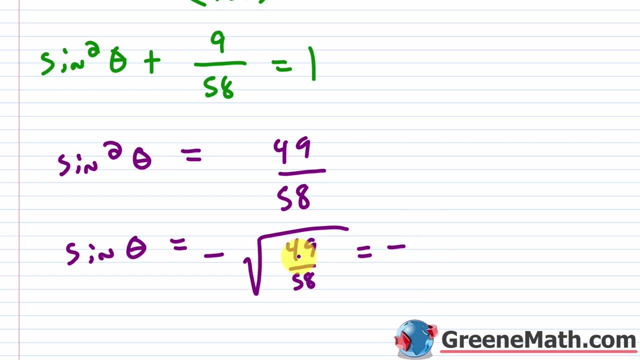 this is equal to the negative of you have. the square root of 49 is seven. So we'd have seven up here over. you'd have the square root of 49 over 58.. So you'd have the square root of 49 over 58.. 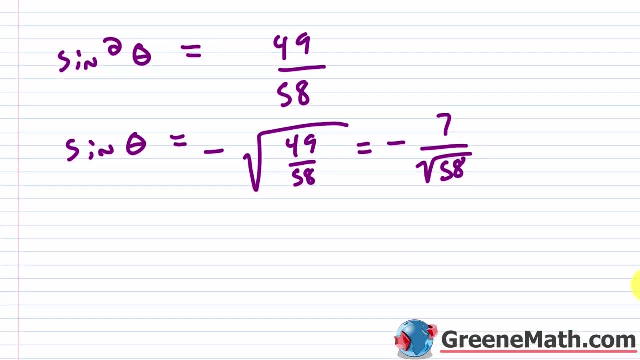 And to make this a little bit cleaner, because again we want to rationalize, the denominator Sine of theta is going to be equal to: you have the negative of seven times the square root of 58 over 58, right, Because I'm going to multiply this by the square root of 58 over the square. 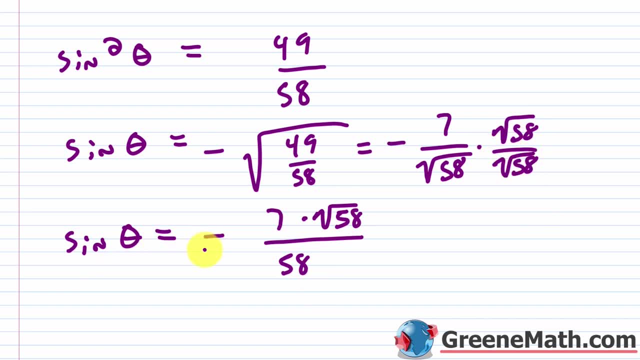 root of 58, and I'll be done So. sine of theta is equal to negative of seven times the square root of 58 over 58.. All right, So let's take a look at another example. We want to find sine of theta. 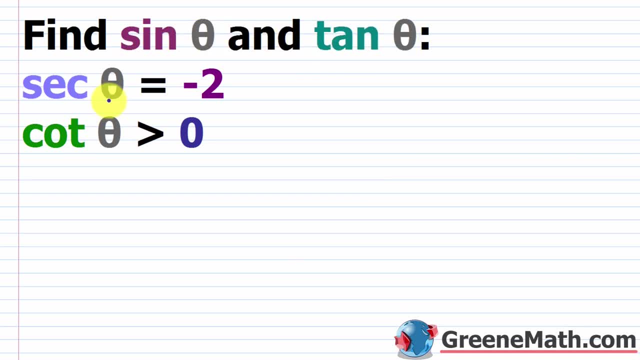 and tangent of theta, Given the fact that the secant of theta is negative, two and the cotangent of theta is greater than zero, or you could say, positive. So the first thing is, what quadrant are we going to be in? Well, where's the secant of theta? negative, It's going to be negative in quadrants. 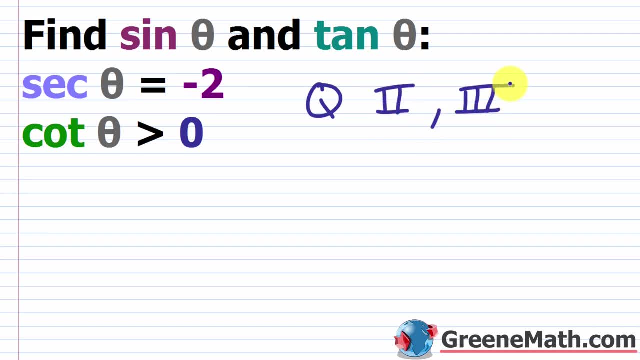 two and also three, Okay, And then where's cotangent of theta? Where is that positive? It's positive in quadrants one and three. Okay, So three matches, both conditions there. So we'll say this is in quadrant three. Okay, So this is going to be in quadrant three, And then we're 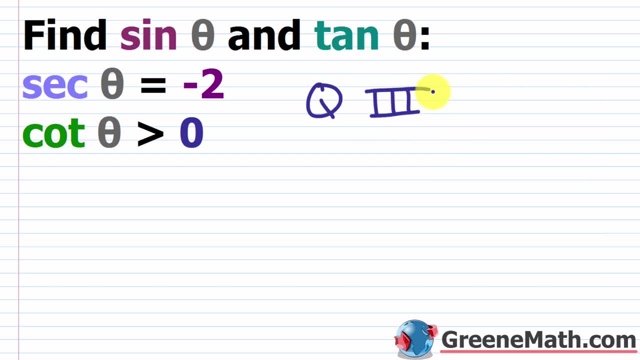 going to be in quadrant three. So when we look at this, we know that our sine of theta will be negative and our tangent of theta will be positive. Okay, So keep that in mind when you're solving this problem. So the first thing is we're given the secant of theta is negative two. So 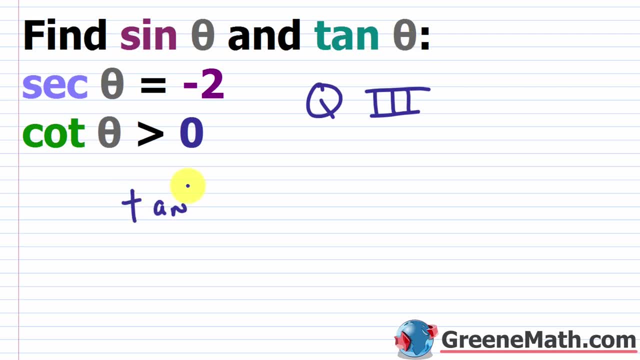 let's plug in to this guy. We have the tangent squared theta plus one is equal to the secant squared theta. So I'm just going to plug in for this. Remember it's squared, So it would be negative two squared, negative two, both the negative and the positive. So we're going to be. 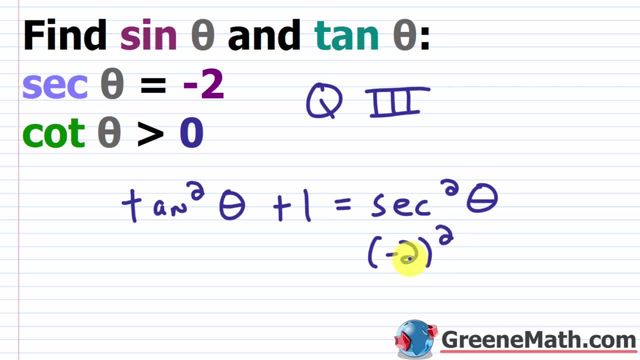 and the two being squared. If I did that, that would be positive four. So let's just erase this and put four in here. Okay, I'm going to subtract one away from each side of the equation, So this is gone and this would be a three. So what you have here is tangent squared. theta is equal to. 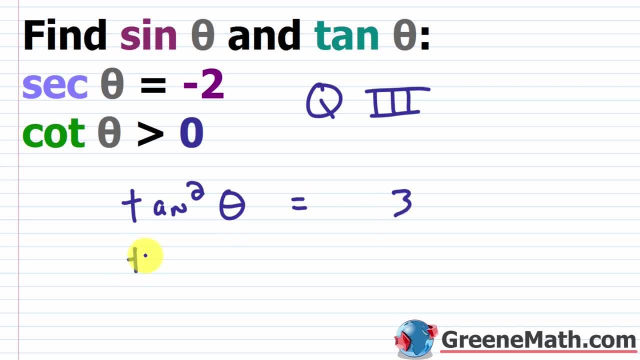 three, If I want to find out what tangent tangent of theta is, I'm going to take the square root of each side. Remember, we already said this guy's going to be positive, So I don't need the plus or minus, I just want the principal square root here. So it's just the principal square root of. 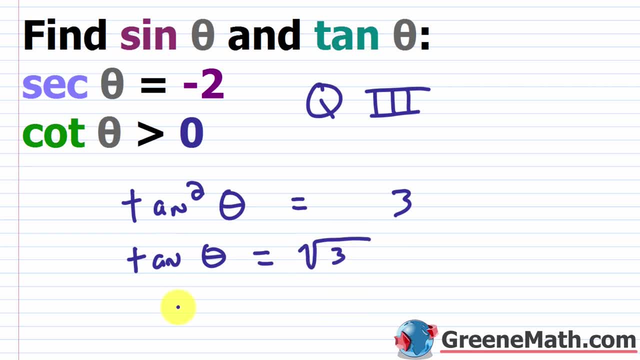 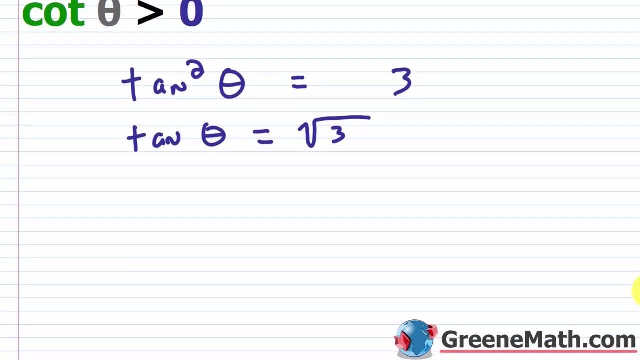 three. Okay, So that's my tangent of theta. So now that we know what the tangent of theta is, how can we find the sine of theta? Well, one thing we can do: we can flip this guy. Since the tangent of theta and the cotangent of theta, those guys are reciprocals, I can say my: 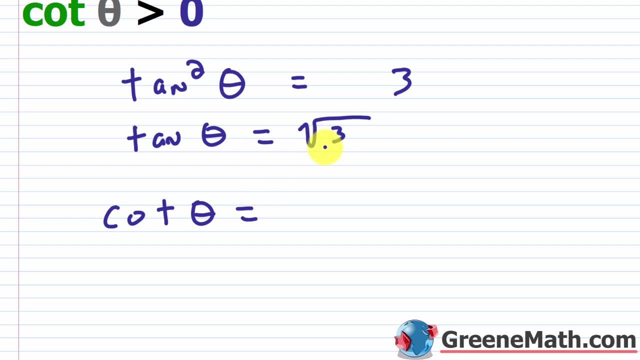 cotangent of theta is just flipping this guy. Remember, if it's not displayed as a fraction, just write it over one and then flip it So you can say this is one over the square root of three. We're not going to rationalize this here because it's not going to be our final. 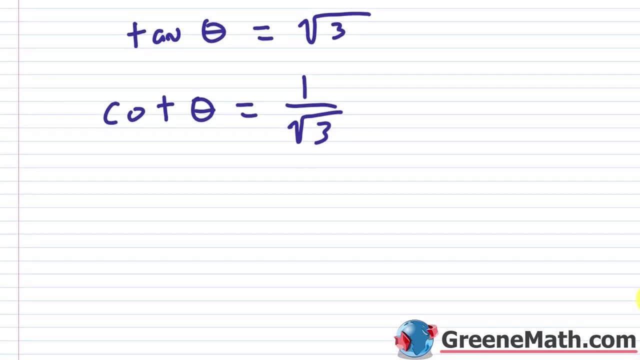 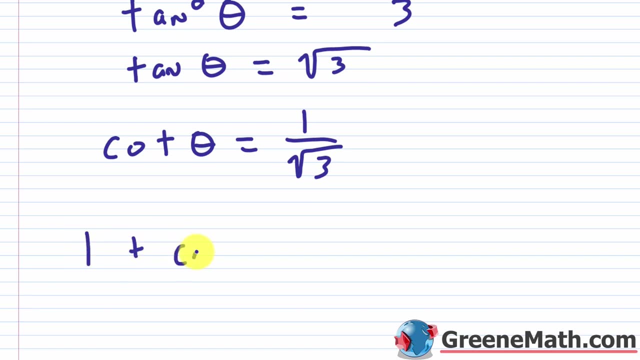 answer. So what I'm going to do now is I'm going to plug this in. I'm going to plug this in for our Pythagorean identity, where it says: one plus our cotangent squared theta is equal to cosecant squared theta. Remember the cosecant of theta and the sine of theta? those guys are reciprocals. 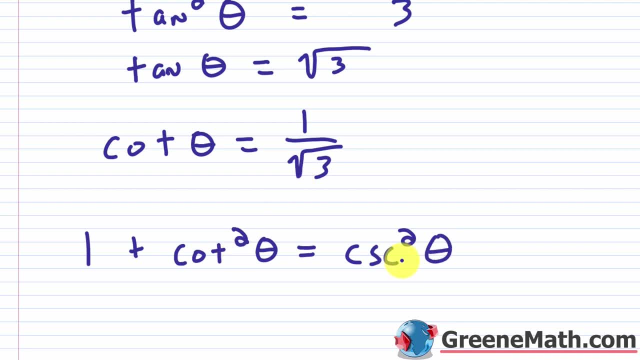 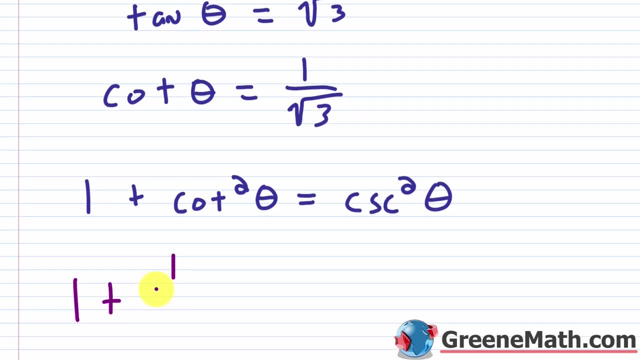 So I can plug in here, find out what this is, flip it Okay And I'll have sine of theta. So let's go through and plug in One plus. I'm going to plug this guy in here. one over square root of three. 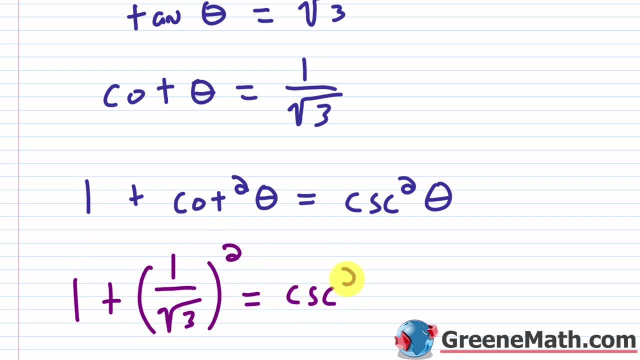 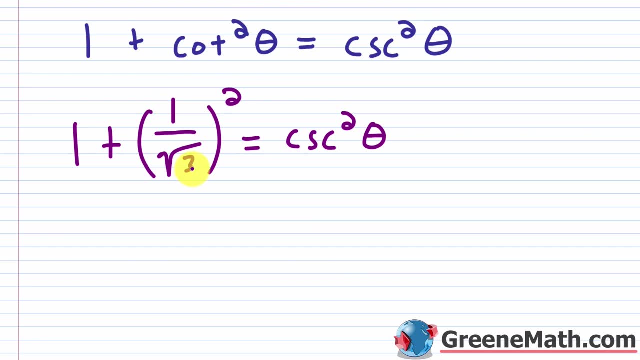 This guy's going to be squared And this equals my cosecant squared theta. Okay, Let's get some room going, And so now, if I square this, I'm going to get what I'm going to get. one squared is one, square root of three squared is three. So this is just one third. This is just one third To add. 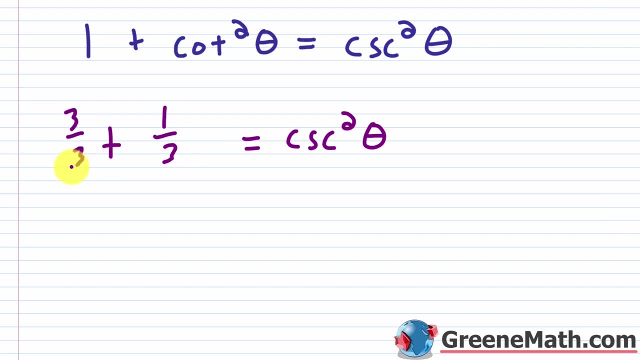 this to one, I'm going to get a common denominator and say: this is three over three. So this is basically going to give me four thirds. So four thirds is equal to- and let me write this in another way: So cosecant squared theta is equal to four thirds. Okay, So to solve for. 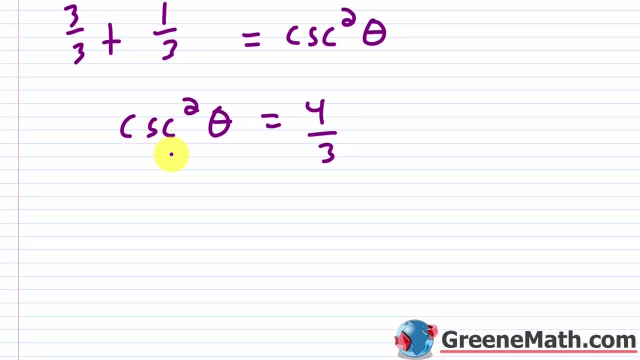 this guy, remember. the cosecant in quadrant three is going to be negative. So I'm going to take the square root of this side. I'll say the cosecant of theta is equal to over. here I want the negative square root of four thirds. So the cosecant of theta is going to be the negative of the square. 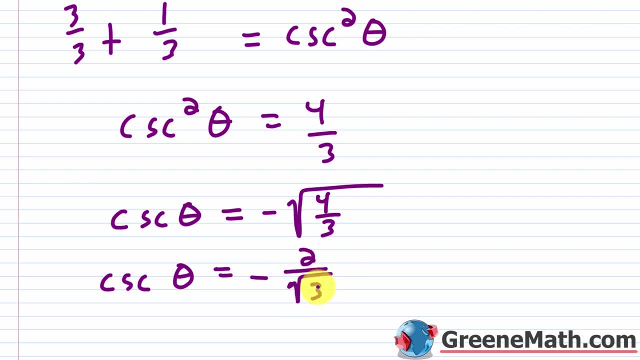 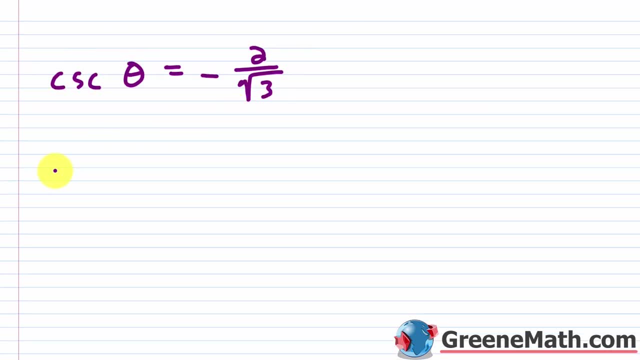 root of four is two And then over the square root of three. So now let's cut this. We'll go to a fresh sheet and we'll just paste this in right here. So remember, if I want the sine of theta, I just flip this guy. Okay, So if I flip this guy, I'm going to have the negative of 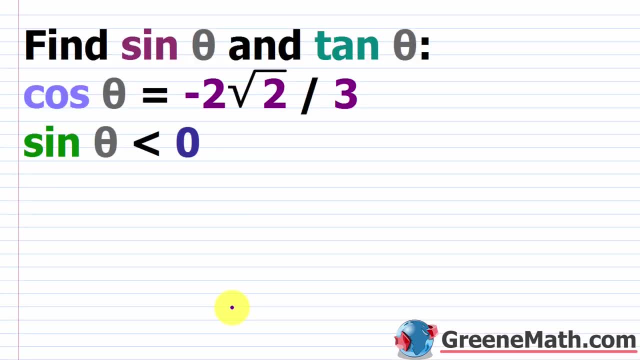 the square root of three over two, And that's my answer. All right, Let's look at one that involves the quotient identities. So we have find sine of theta and tangent of theta, given the fact that our cosine of theta is equal to negative two times square root of two over three. and sine of 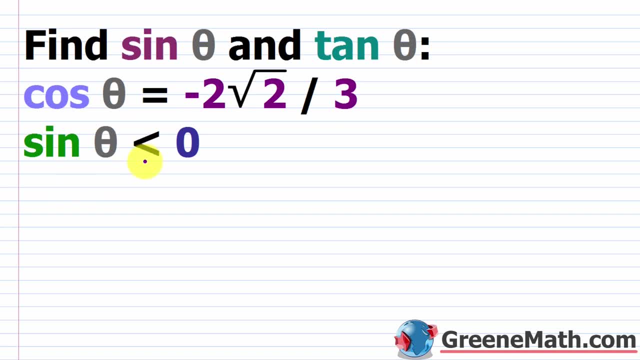 theta is negative. So cosine of theta is negative here. Where is cosine of theta negative? Well, it's negative in quadrants two and three. Where is sine of theta negative? It's negative in quadrants three and four. So again we have a situation where we're in quadrant three. Okay, And it doesn't always. 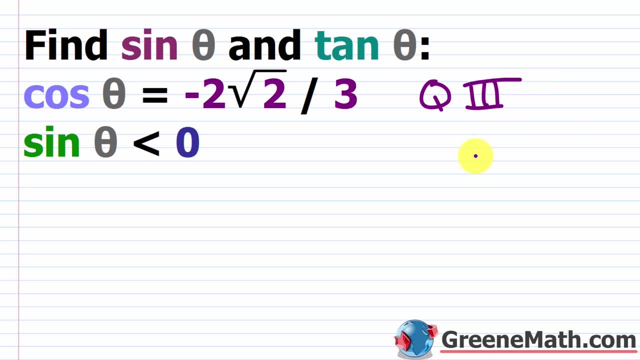 work out this way. We had three problems today where they're all in quadrant three, but it's going to vary based on the problem you're given. So we know we're in quadrant three From here. we're going to say that. we know we're in quadrant three. So we're going to say that we know we're. 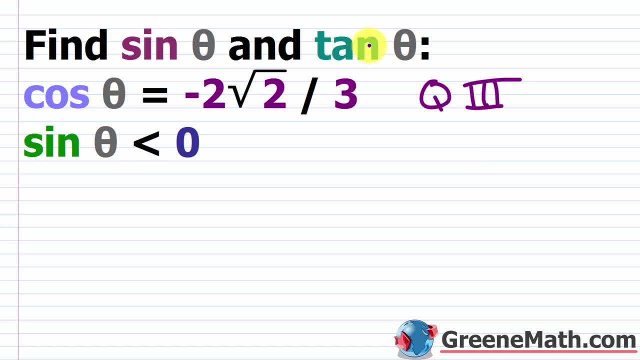 in quadrant three. We know our sine would be negative. It's given to us And we know our tangent is going to be positive because we're in quadrant three. Okay, So how do we find our sine of theta? Well, we can use our Pythagorean identity, the one that says cosine squared theta. 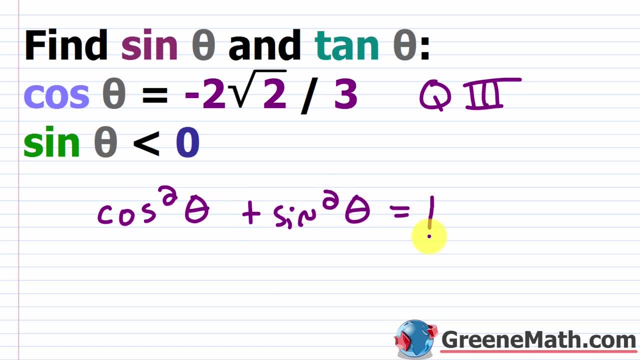 plus sine squared theta equals one, And I know this is normally reversed, but I'm writing it this way to give myself some room, because I want to plug in here, So I'm going to plug in. I'm going to plug in for cosine theta, Okay. So I'm going to say this is negative And I'm going to. 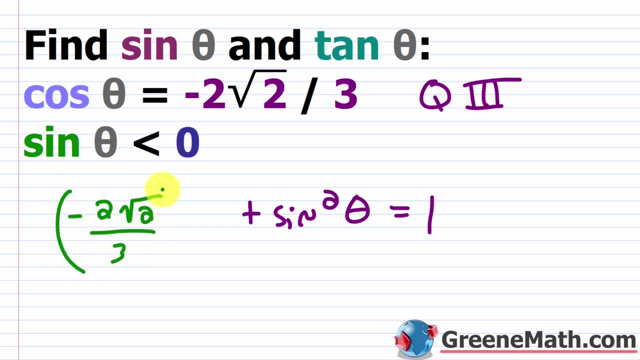 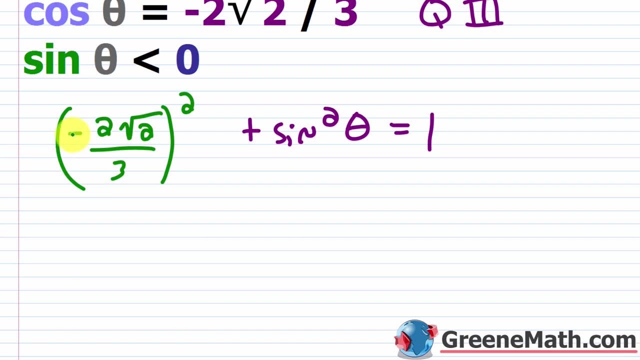 say negative two times the square root of two over three. Remember, this guy is squared. It's so important that you don't forget to square things, Okay? So if I square this guy, the negative becomes positive. So you can forget about that. Two squared is four. The square root of two squared. 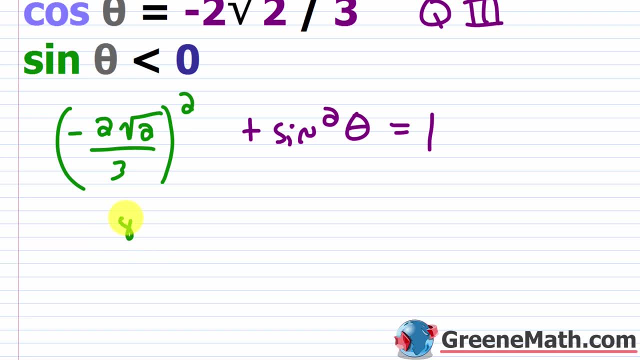 is two. Okay, Four times two would give me eight, And then down there you have three, which is squared, which is not, So I have eight. ninths plus sine squared, theta equals one. Okay, Let me erase this. We're just going to kind of stick around here, because I'm going to need some of that. 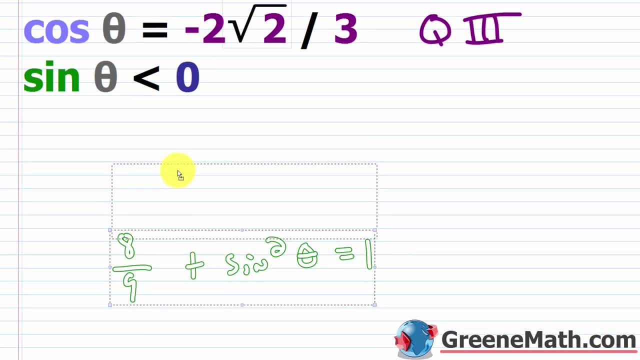 information. So I'm going to be going back up, So let me just kind of drag this up a little bit so that we stay right here. Okay, So what I'm going to do now is I'm going to subtract eight ninths away from each side, So I'm just going to erase it from over here. I'm going to write this: 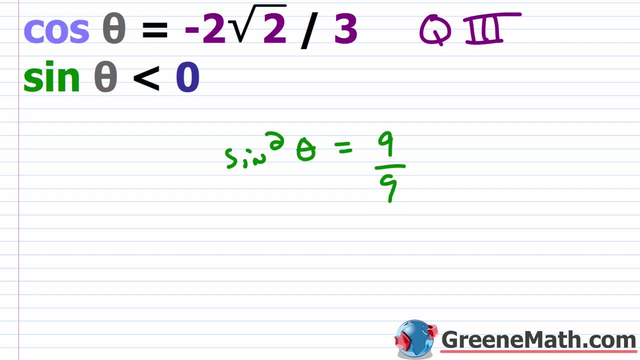 as nine ninths. So I have a common denominator and then we're going to subtract away that eight ninths, Okay. Nine ninths minus eight ninths is one ninth, Okay, So one ninth. Remember, sine of theta is negative. So if I take the square root over here, I want sine of theta is equal to: 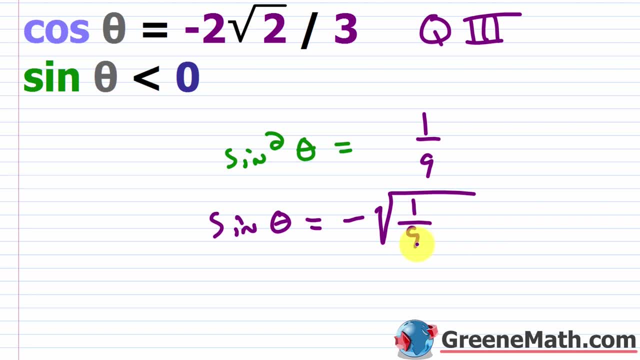 one ninth. Now, the square root of one ninth is the square root of one, which is one, over the square root of nine, which is three. So it's one third, right. So this is negative one third. negative one third, All right. So let me erase this real quick. I'm just going to drag this over here. 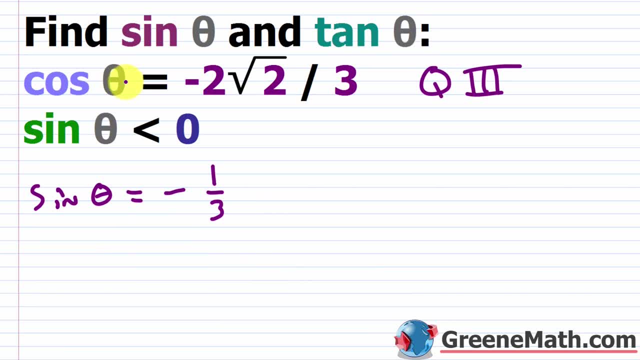 And I want to find tangent of theta. Now, given the fact that I know what cosine of theta is, I know what sine of theta is. Remember, the tangent of theta. the tangent of theta is defined as the sine of theta divided by the cosine of theta. So I'm going to take the sine of theta and I'm going to 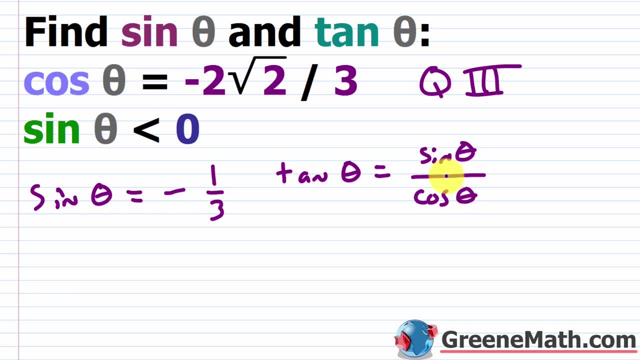 take the cosine of theta, Okay, So what I can do- it's going to be hard to fit this in this limited room- I have- but I would have that- the tangent of theta. let me just write that over here. So the tangent of theta is equal to the sine of theta is negative, the negative of one third divided by the. 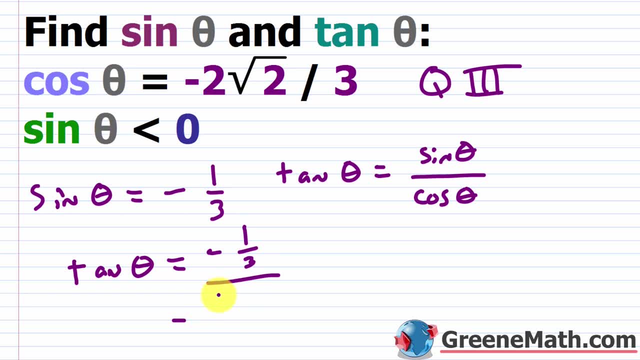 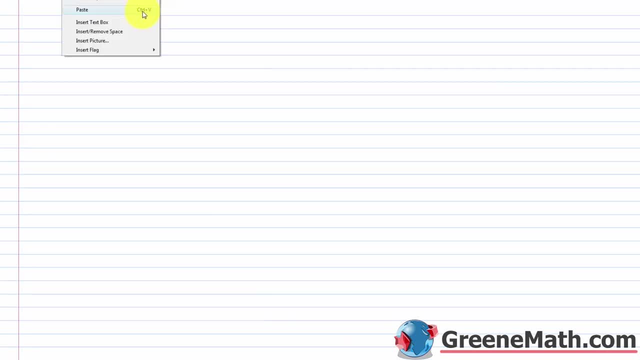 cosine of theta, which is the negative of two times square root of two over three. So let me just copy this and we're going to go to another sheet. We'll paste this in here real quick. So this is equal to what? It's equal to the negative of one third times. flip this guy. the negative of 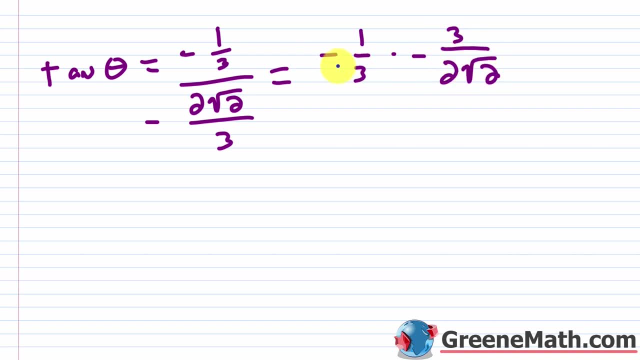 three over two times square root of two. Of course, the negatives are going to cancel. Forget about those. The threes are going to cancel. So what I'm left with here is one over two times square root of two. Let's rationalize: We're going to multiply by square root of two over square root. 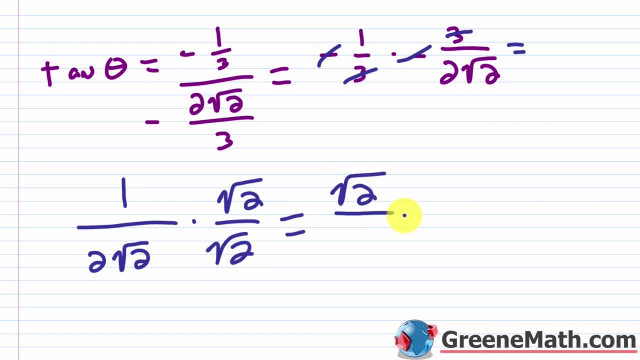 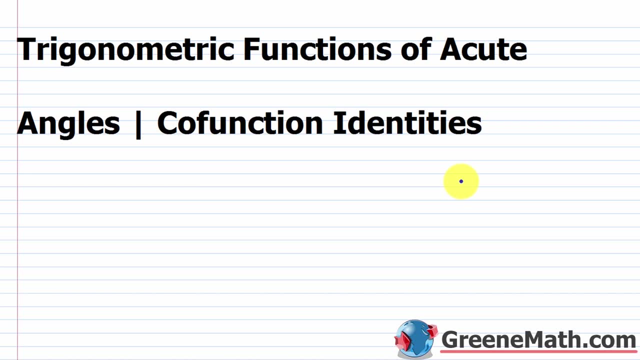 of two, And this gives us the square root of two over square root of two times square root of two is two. two times two is four. So square root of two over four would be your tangent of theta. In this lesson we want to talk about trigonometric functions of acute angles. 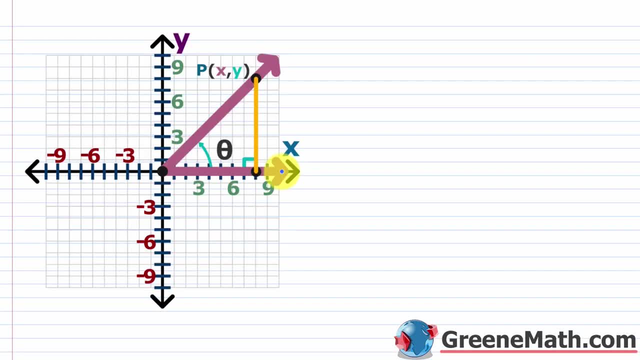 And also we'll look at co-function identities. So previously we used angles in standard position to define the six trigonometric functions. So what we're going to do in this lesson is we're going to define our six trigonometric functions as ratios of the lengths of the sides of right. 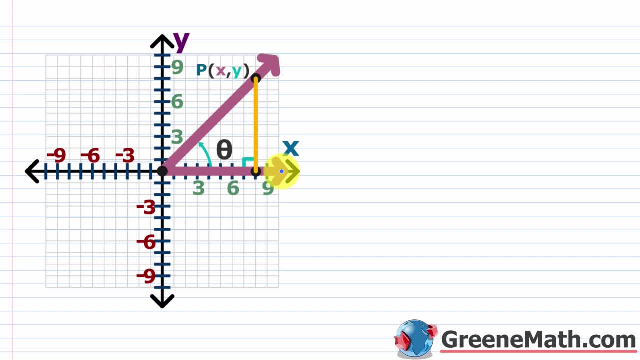 triangles. So we're going to kick things off by looking at an acute angle in standard position. This is something we've already seen, So we've seen this diagram before. So this acute angle here, this angle, theta, is in standard position And we've just picked a point on the terminal side. We're going to call. 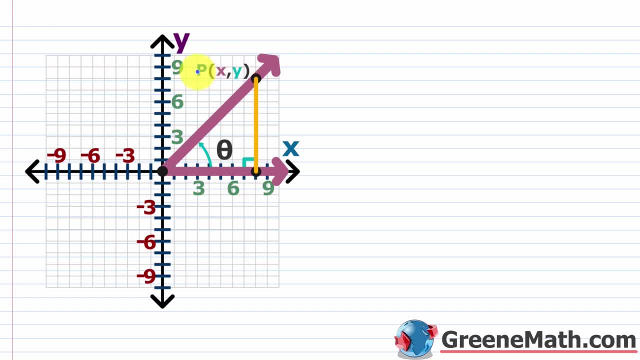 it x comma y. That's our point. But again, this has actual coordinates. In this case it would be eight comma eight, But we're just going to refer to it as x comma y. Now, generically we know that. 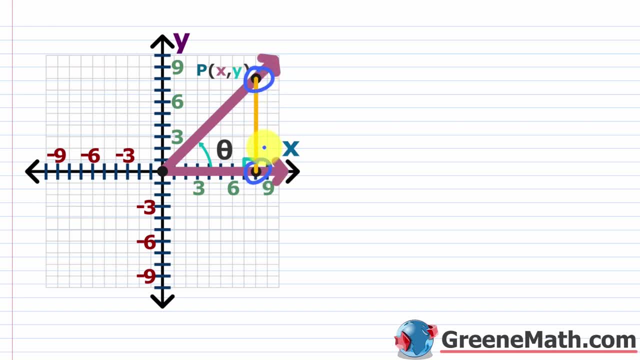 this distance from here to here can be represented by just saying the letter y, Because this right here is y And down here this coordinate is going to be zero Because we're on the x-axis. So I could take y and subtract away zero and I would get y. So that's my distance for this. 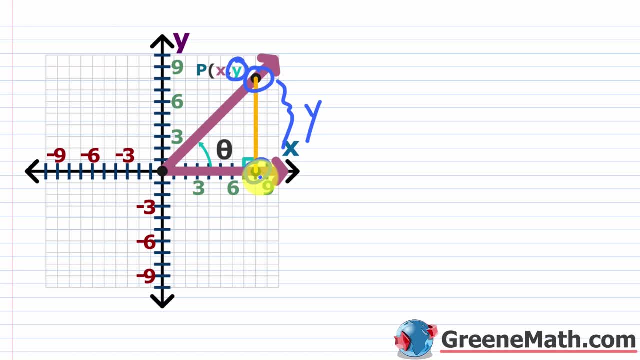 vertical leg here, of this right triangle that we formed. Then this horizontal distance from here to here- Remember, this is a coordinate of x, This is a coordinate of x And this is a coordinate of zero. So really I could do x minus zero And just say that the distance 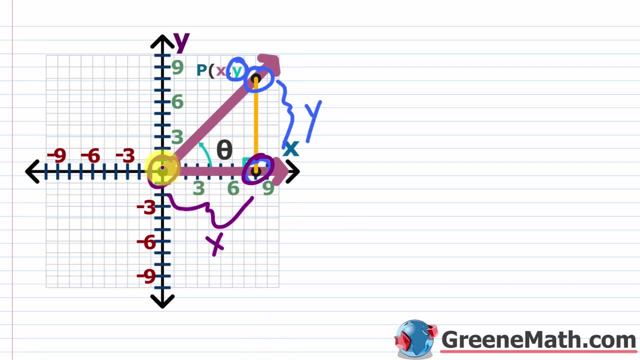 from there to there, we could say: this is x. Okay, Then from here to here- let me highlight this: From here to here, we know that is the hypotenuse right, So we call this r, We call this r. We'll get more into that as we progress. 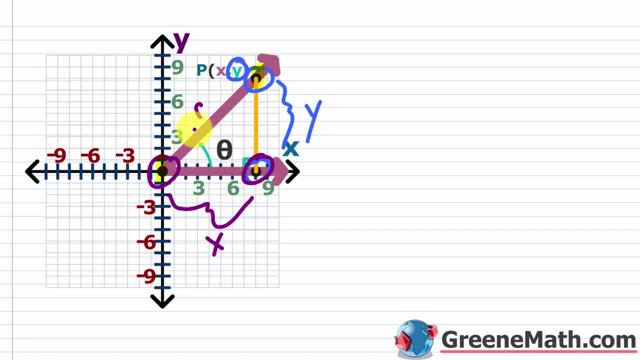 through the course in terms of why we call it r, But right now we just call it r. Okay, So we've already defined the six trigonometric functions using these letters, right? So we've said that the sine of theta is y over r. We've said that the cosine of theta is actually the cosine of theta. 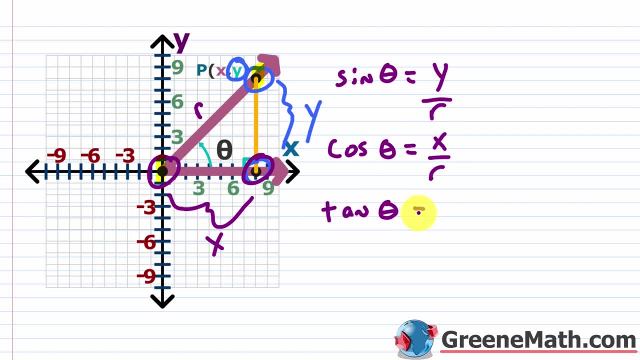 x over r. We've said that the tangent of theta is y over x And then, using the reciprocal identities, we can get the three remaining ones. So the cosecant of theta is going to be the reciprocal of this, which is r over y. And keep in mind if your denominator ends up being: 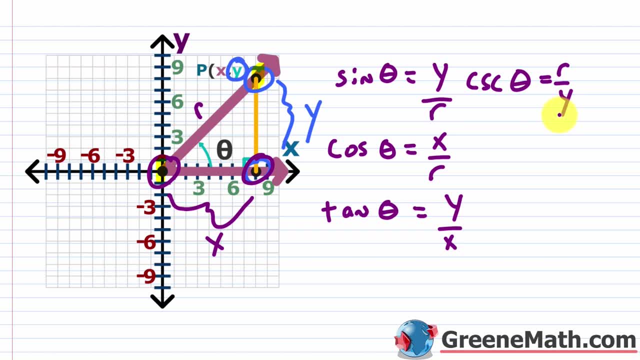 zero. okay, it's undefined, So I'm not going to write that. but y can't be zero there. Then here you would have the secant of theta, Okay, And this would be r over x, And then last. 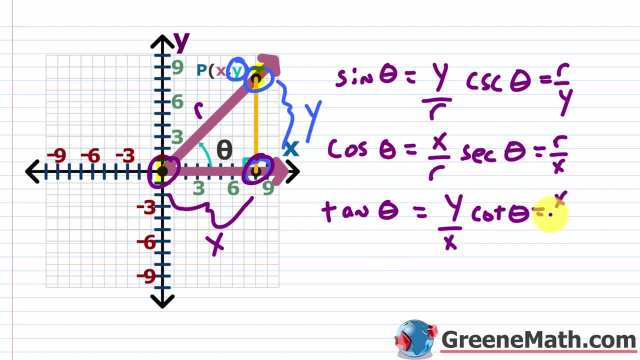 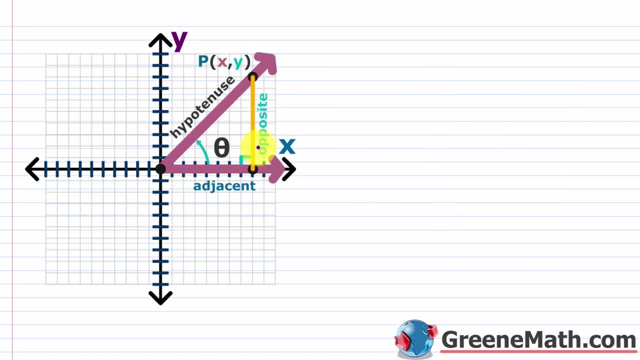 you'd have your cotangent of theta, which is going to be x over y, Okay, so let's explore a different way to look at this now. So instead of calling this guy y, okay, we're going to refer to it as opposite, because it's opposite of this angle here. Okay, Now, what you want to pay attention to. 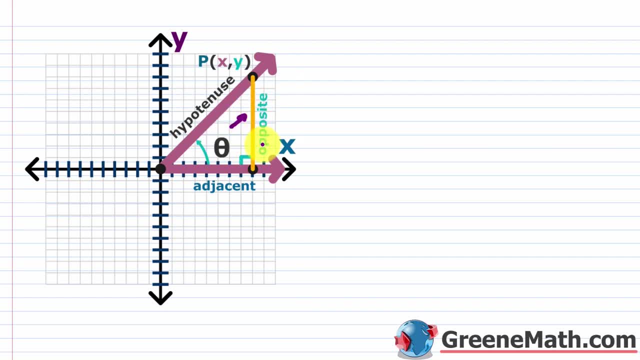 is where this guy is, because in this case this is the opposite side. But if I change the angle up, if I was measuring this angle here, well then the opposite side would now be here. So you got to pay close attention to this. I'll show you how to do that in a minute. So let's go ahead and 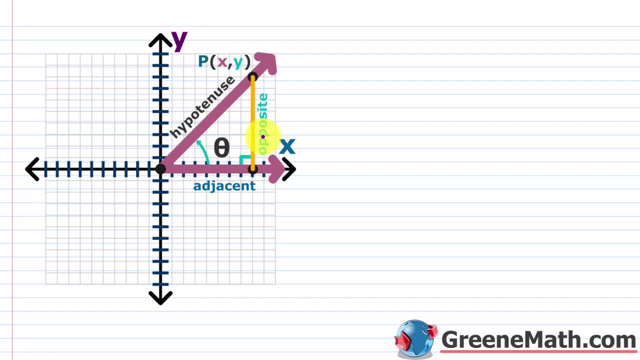 show you some examples where we switch things up and the answers are going to change. So you got to keep in mind where the opposite side is. So this guy is opposite of your angle, theta, And then this guy right here is adjacent to it, Okay. And then, of course, the hypotenuse stays the same, The 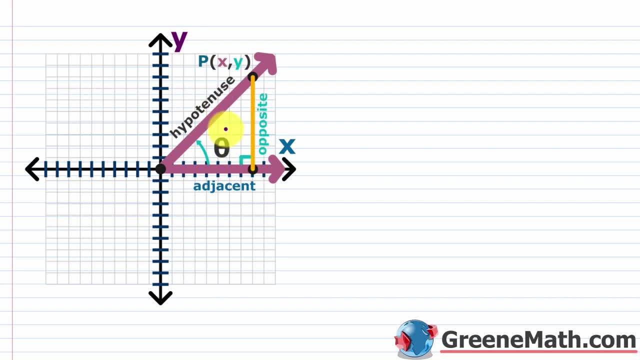 hypotenuse is always opposite of your right angle, your 90 degree angle. Okay, So what we can do now is say that, okay, since this was y and this was x before and this was r. well, if we have sine, 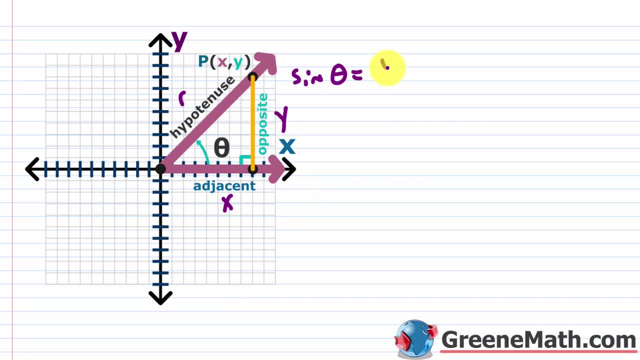 of theta. okay, we said before this was y over r and this was y over r and this was y over r. Now we're going to say: it's what? Well, y is the opposite. So I'm going to put OPP for opposite. 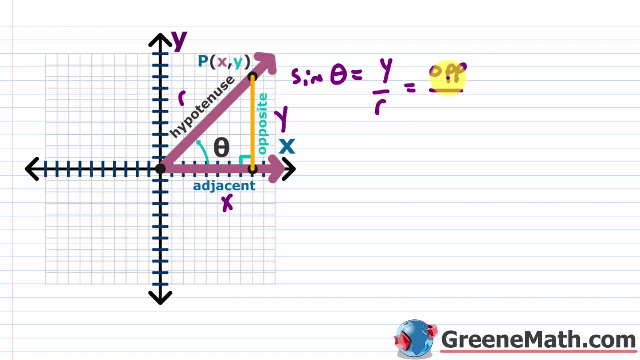 And this again is the measure of that, So the length that you're given. And then you have your r, your hypotenuse. So I'm going to put HYP for hypotenuse, So opposite over hypotenuse. Okay, 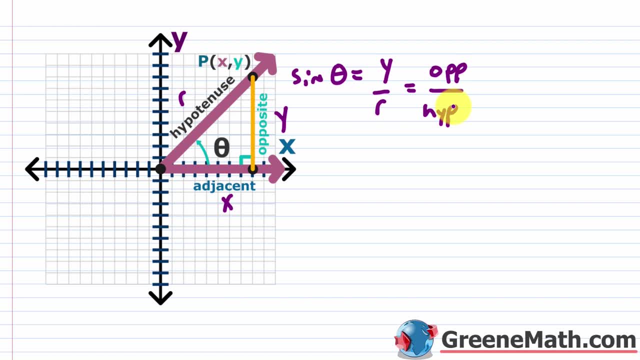 And I'll give you a mnemonic device for this in just a moment, the SOHCAHTOA. So then you have your cosine of theta. Okay, This is x over r, Or, in terms of this, it's the adjacent. Okay, The. 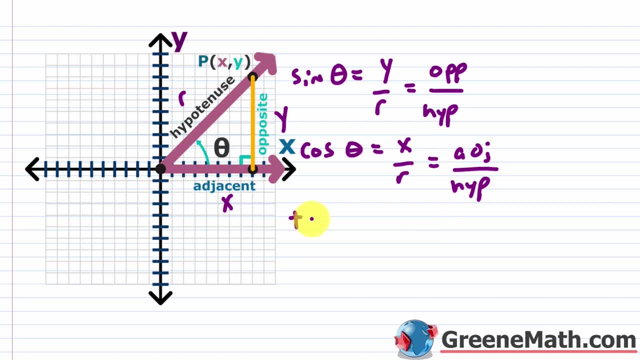 adjacent, over adjacent. And then you have your cosine of theta: Okay, This is x over r. And then you have the hypotenuse, Okay, And then you have your tangent of theta, which is going to be what It's: y over x, which is your opposite. Okay, Your opposite over your adjacent, Over your adjacent. 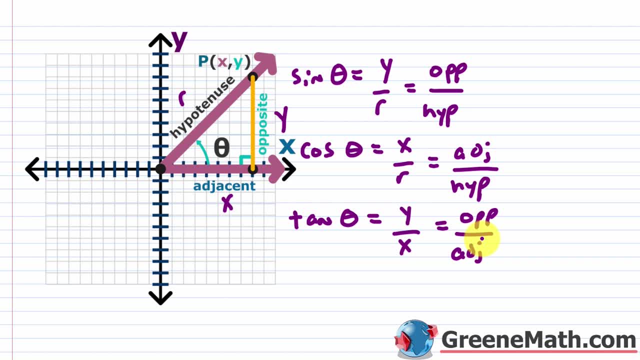 And then, of course, you can flip these guys and you can get your cosecant of theta. So your cosecant of theta, And I'm going to run out of room here, So let me actually copy this real quick And let's go to a fresh sheet. 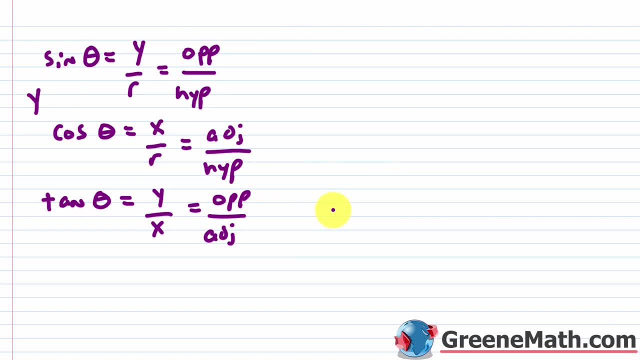 And just paste this in So we have more room. So then I can say that cosecant of theta, which is the reciprocal of this, is going to be the hypotenuse over the opposite, And then your secant of theta, which is the reciprocal of this, would be your hypotenuse over your adjacent. 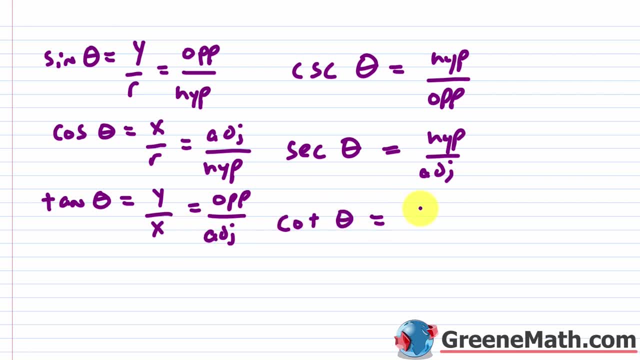 And then, lastly, your cotangent of theta is going to be the adjacent over your opposite. Okay, So how do we remember this? Well, recall, when you work with something like the order of a constant, you have your PEMDAS right, Your, please excuse my dear Aunt, Sally. Well, you have a similar. 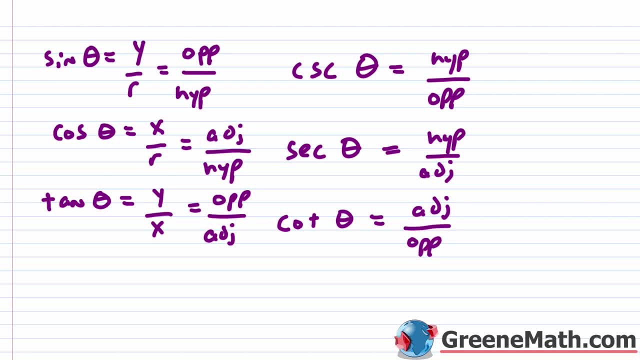 mnemonic device. here It's the SOHCAHTOA. Okay, So the SOHCAHTOA. Okay, So the S stands for sine, the C stands for cosine and the T stands for tangent. Okay, So this is pretty much what. 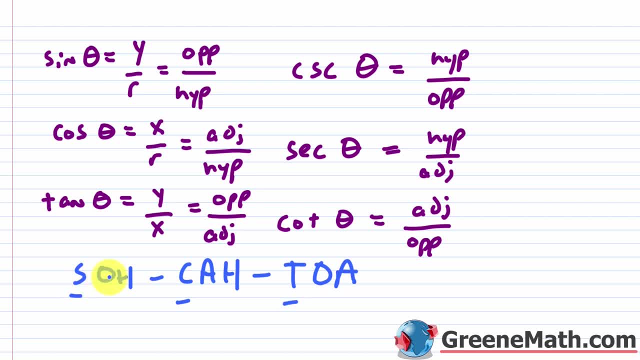 everybody uses to remember these guys. So S for sine, it's the opposite over the hypotenuse, So opposite over hypotenuse. C for cosine, the adjacent over hypotenuse, So the opposite over hypotenuse, So adjacent over hypotenuse. The T for tangent, the opposite over adjacent, So opposite over. 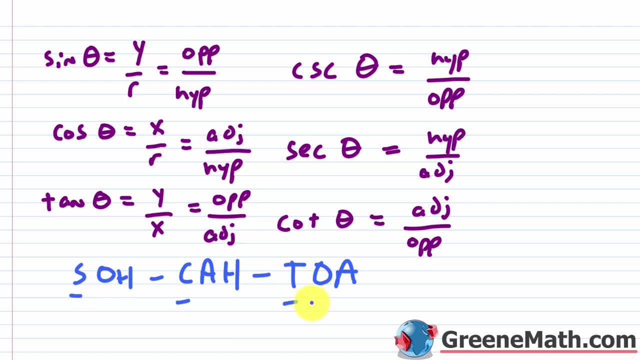 adjacent, So this is something you want to write down and think about constantly until you have it memorized. It's going to save you a lot of time. And then, of course, if you know your reciprocal identities, it's very easy to get the cosecant, the secant and the cotangent by just flipping. 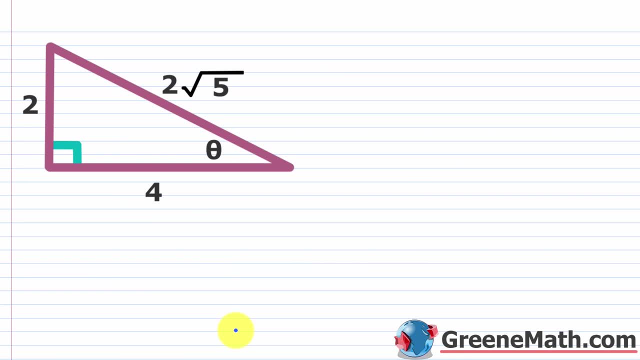 guys. All right, So let's go ahead and take a look at an example. So with this guy right here, we're just going to find the six trigonometric functions. So let me just write them out. We want sine of theta, cosine of theta and let's just do tangent of theta. for right now We know we can get. 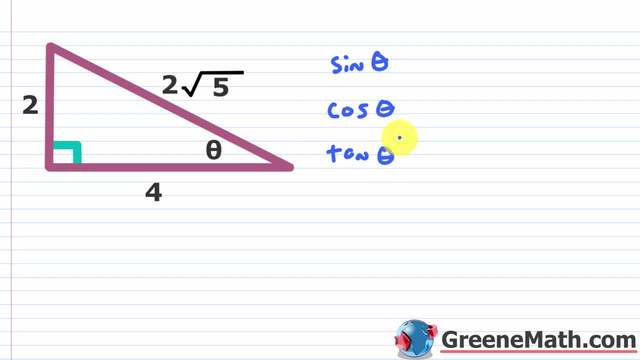 the other three by just flipping these guys. Okay, So what is sine of theta? Again, let me go back to the so-ca-oa. Okay, So, sine of theta, it's Y over R, but let's think about it in terms of this: 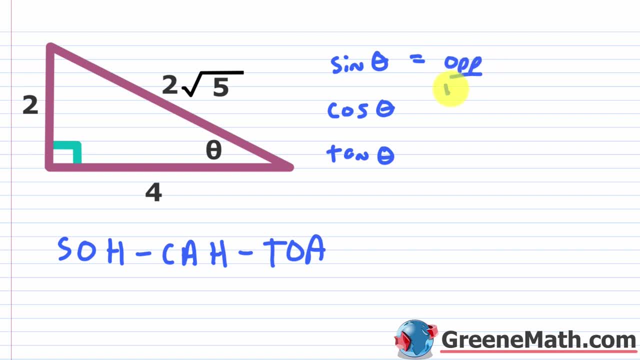 We're going to say opposite, So opposite over hypotenuse. Okay, Cosine of theta, we're going to do the opposite, the opposite over the adjacent, Okay. So what's the opposite here? What's the hypotenuse, What's the adjacent? So we know that across from the right angle, 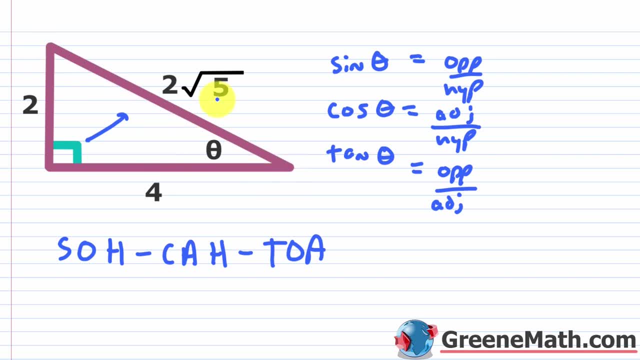 okay, which is the longest side of a right triangle is your hypotenuse? Okay? So this is the hypotenuse right here. Okay, And if you're confused about these things when you first start, go ahead and take the time to label things, figure out where everything is. 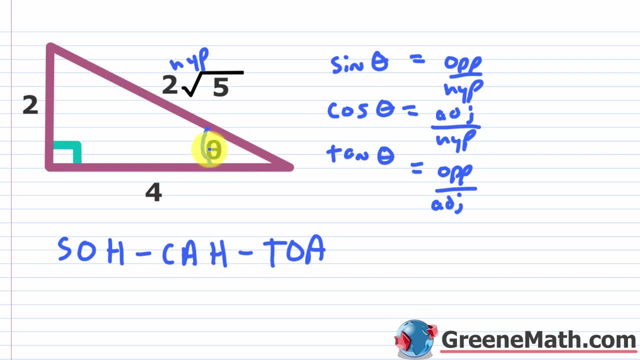 So this guy right here is adjacent. This is your angle here, theta. Okay, And I made that terribly. So this is your angle here, theta. This guy is adjacent to this, Okay, Or next to it. So this is going to be your adjacent, your adjacent, And then opposite of this you're. 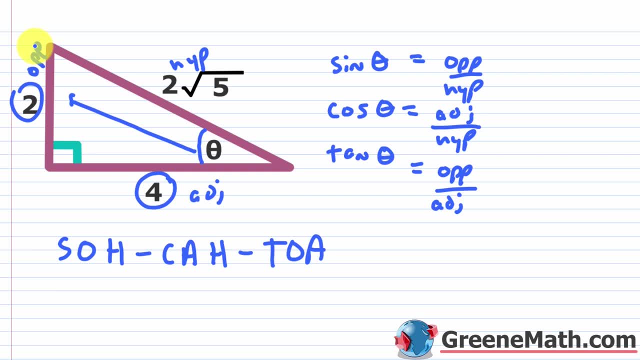 going to have this guy right here. So this is your opposite. Once you've figured this out, you're just plugging things in and you're done. Okay, That's all you need to do. So what is the opposite? It's two. What is the hypotenuse? It's two times square root of five. 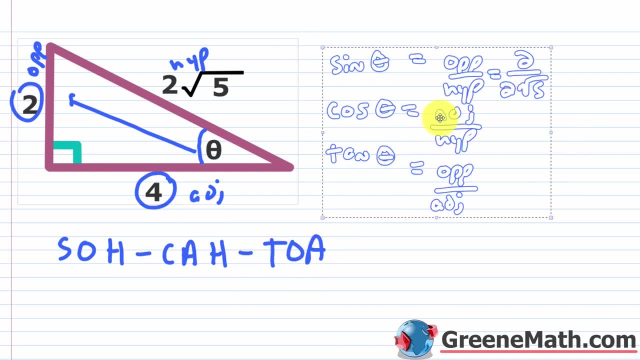 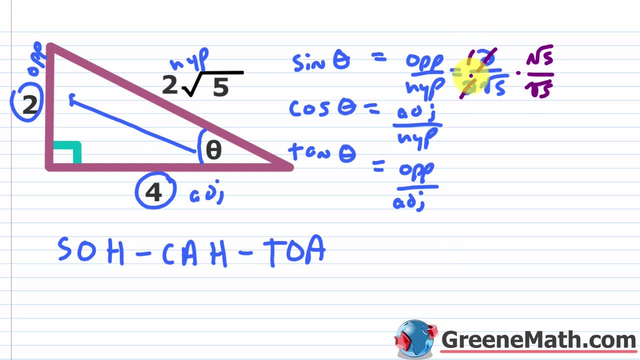 Of course you want to rationalize the denominator there. Let me just kind of scooch this down a little bit So we have some room. So I'm going to multiply this by square root of five over square root of five. The twos are going to cancel, So I'm going to have the square root of five over. 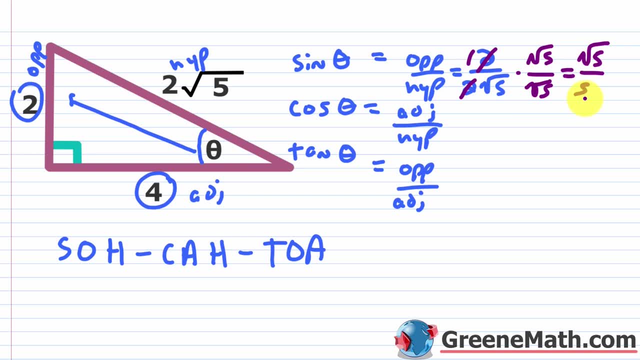 square root of five times square root of five is five. Okay, So that's my sine of theta. My cosine of theta is the adjacent okay, which is four over the hypotenuse, which is two times square root of five. The four and the two would cancel to two up there. So again, you're just going to multiply by. 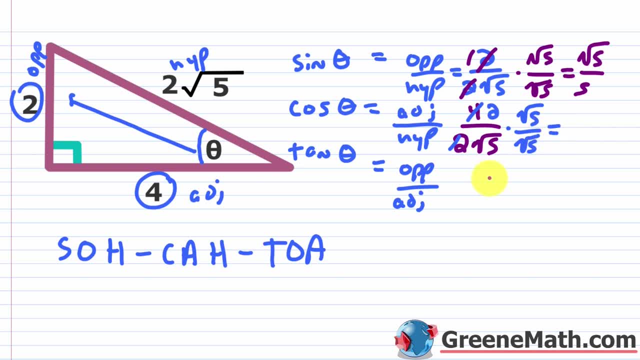 five over the square root of five. And what does that give me? Well, two times square root of five, two times square root of five over square root of five. times square root of five is five. So the last one down here we have the opposite over the adjacent, So the opposite is two The 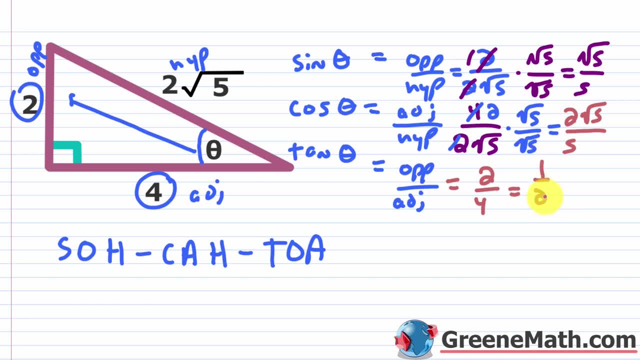 adjacent is four, So this is one half. Now we can flip these guys again and figure out our other ones, So let me erase this, All right. So for the cosecant of theta, remember that's a reciprocal okay, So I'm going to use the one before we rationalize the denominator, to make it easy. So 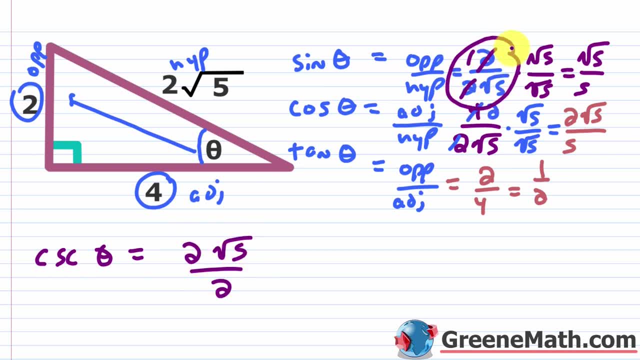 two times square root of five over two. I just took this guy right here, Okay, And I flipped it. That's all I'm doing. You can flip this guy too, but then you have to rationalize the denominator again. It's just double work, Okay, So we've already done that, So cancel this with this. 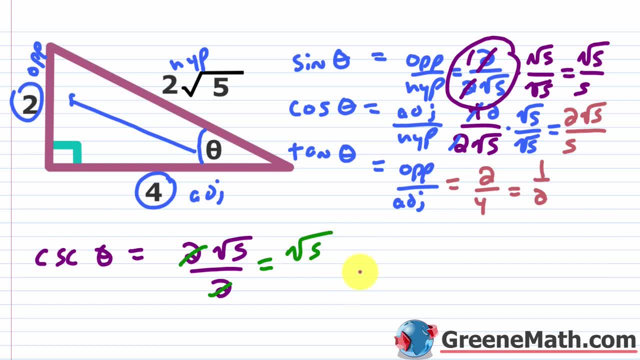 You just get the square root of five, Then the next one. we would have the secant of theta. Okay, And that would give me what The secant of theta would be: the reciprocal cosine of theta. So, again, take the one before we rationalize the denominator, And I'm just going. 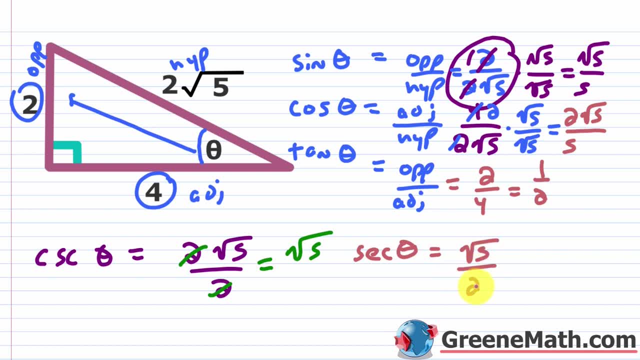 to say: this is the square root of five over two and nothing really else you can do with that. So, lastly, I'm going to flip the tangent of theta- Okay, To get the cotangent of theta. And so if I flip one half, I just get two over one or two, All right. So let's look at another. 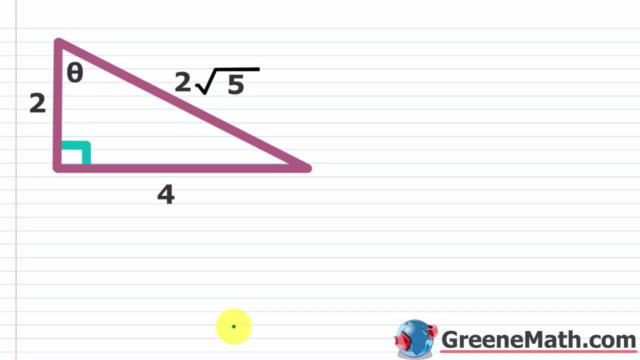 example, We're going to have the same right triangle, but now we're going to change the angle. So before our theta was here, Okay, So we were talking about in reference to that angle. now the angle has changed. Okay, So this is our angle now. And so this guy right. 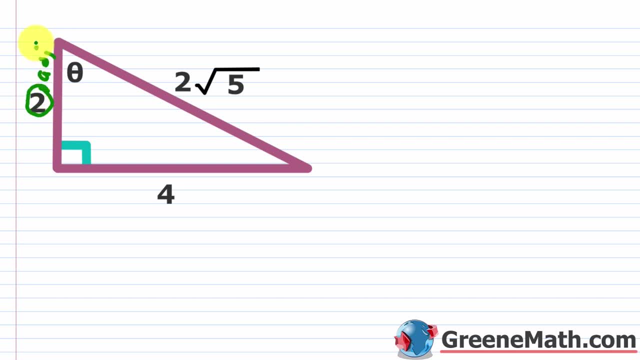 here. now is the adjacent. Okay, So this is the adjacent and this is still the hypotenuse, That is not going to change, because it's always across from the 90 degree angle or the right angle. And now, if you look opposite of this, this is going to be this side over here. Okay, So we've 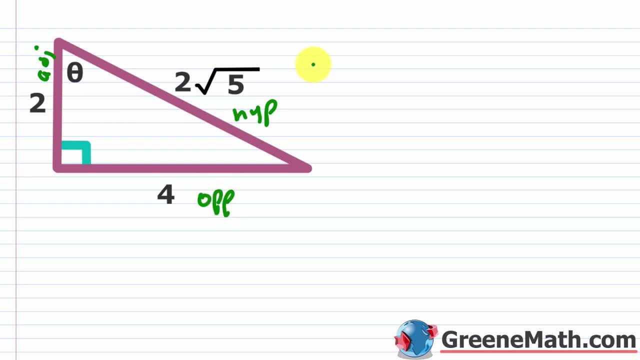 got our adjacent, our hypotenuse and our opposite, So our sine of theta again, so S-O-H. so sine is opposite over hypotenuse. So what's the opposite? It's four. What's the hypotenuse? 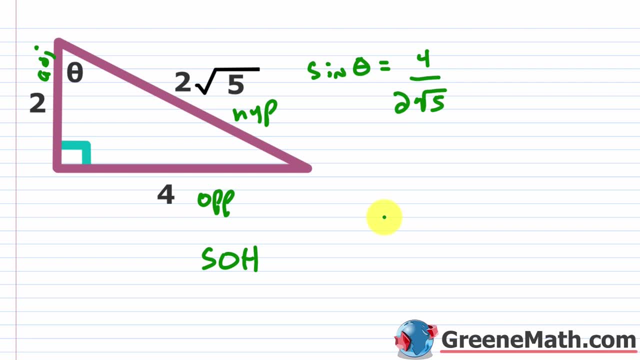 It's two times the square root of five. You do need to rationalize the denominator here, So let me cancel this with this and get a two here. Okay, So two over the square root of five. so this is multiplied by the square root of five over the square root of five, And you're going to 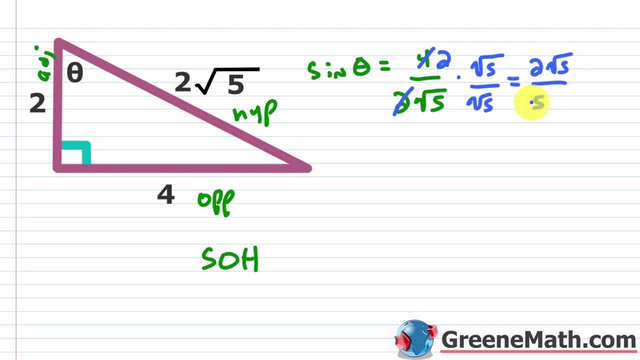 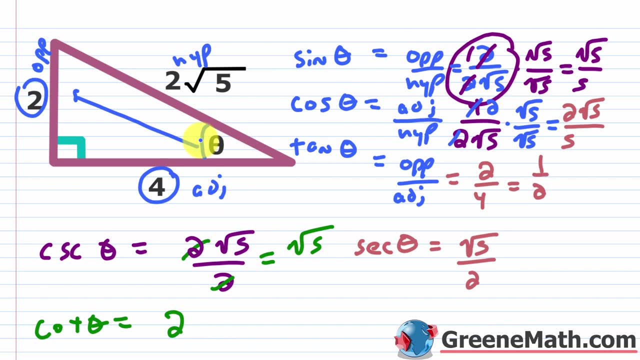 get two times the square root of five over five. Now I want you to notice something: Sine of theta here is the same as cosine, Sine of theta here. Okay, We're going to talk more about this in a moment, but I just want you. 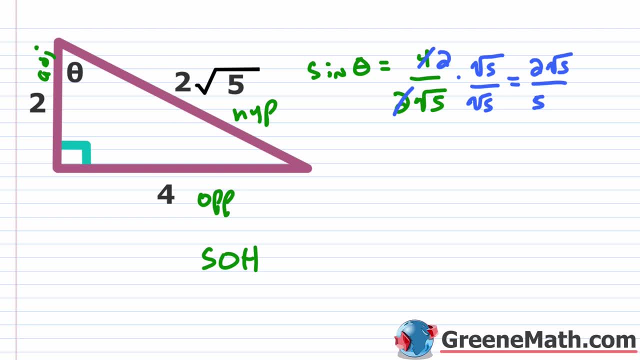 to notice that. All right, So I can flip this guy to get my cosecant of theta. Okay, Let's just do that now, And I'm going to start with it in this form And I'm going to say: this is the square. 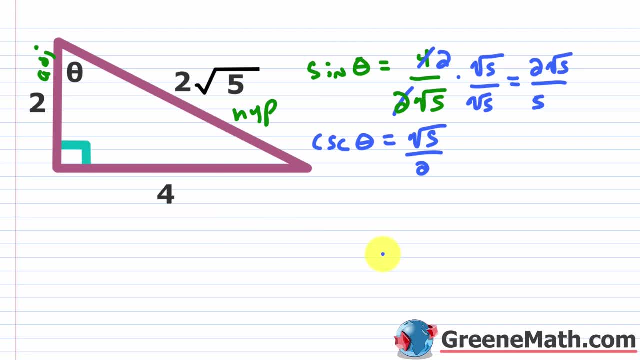 root of five over two. Okay, Let's erase this. So the next one I want, and I'm just going to tighten this down So we kind of make that a little bit neater. So let's move this down a little bit, Okay, So the next one I'm going to do: 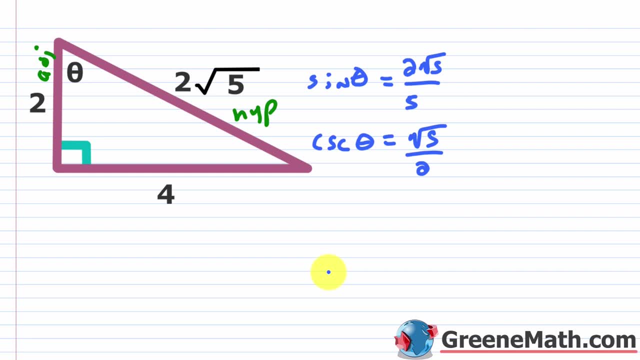 the next one I'm going to do is going to be my cosine of theta. Okay, My cosine of theta. Again, this is the car part of this. So cosine is adjacent over hypotenuse. So where is the adjacent? That's? 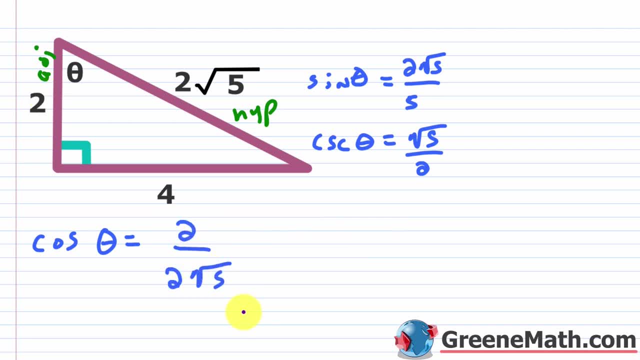 two. What's the hypotenuse? It's two times the square root of five. Before I rationalize the denominator, let's cancel this with this and put a one up here. So this is times the square root of five over the square root of five, And this gives me the square root of five over five. Okay Now. 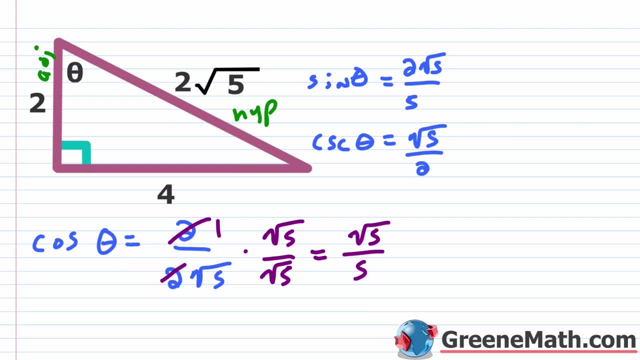 I want you to notice that the cosine of theta here is the square root of five, over the square root of five. Okay, With this angle up there is the same as the sine of theta here. Okay, With the angle here. Again, we'll talk more about this in a moment, So let me flip this guy right here before. 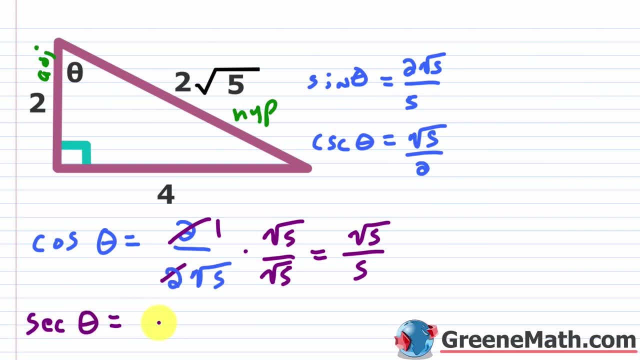 we rationalize the denominator, The secant of theta is going to be the square root of five- Okay, Over one, but just square root of five. So let's just kind of tighten this down a little bit so we don't have stuff all over the place. So let's move this down. And then lastly, 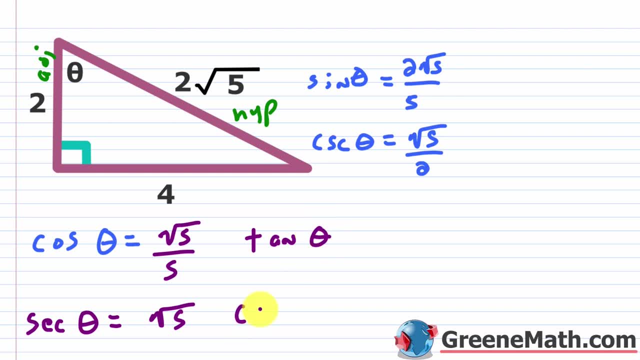 we're going to have our tangent of theta and then our cotangent of theta. Okay, So what's the tangent of theta? That's the TOA part, right? So T-O-A: opposite over adjacent, So the opposite here, and I erased this, I apologize. This is the opposite here. Opposite is four, adjacent is two. 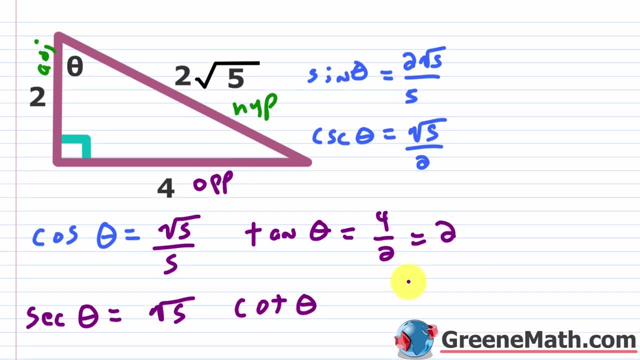 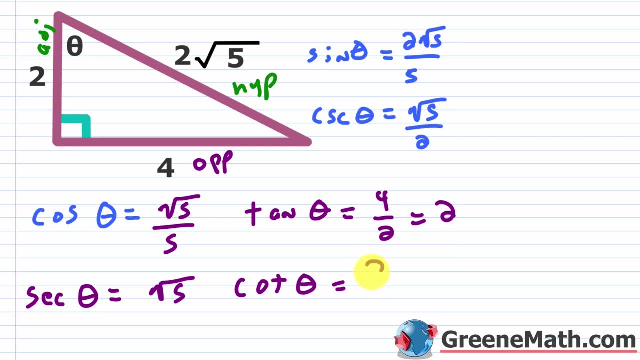 So four over two or two. Okay, And if I flip this guy, remember, if you're flipping a non-fraction number or a whole number, or integer, if you want to think about it that way, you just write the number over one and then flip it right, So it would be one half. So this is one half, And again, 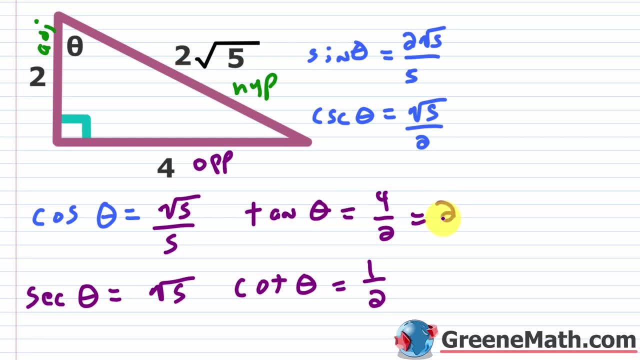 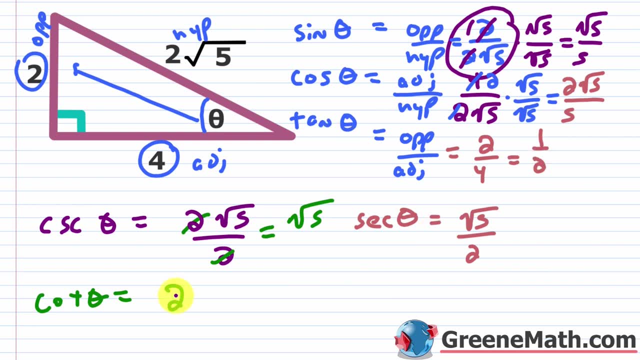 if I look at the tangent of theta here, it's going to match the cotangent of theta here. So the tangent of theta here is a half and the cotangent of theta here is two. Those guys are flipped. So now the tangent of theta is two and the cotangent of theta is one half. So this is: 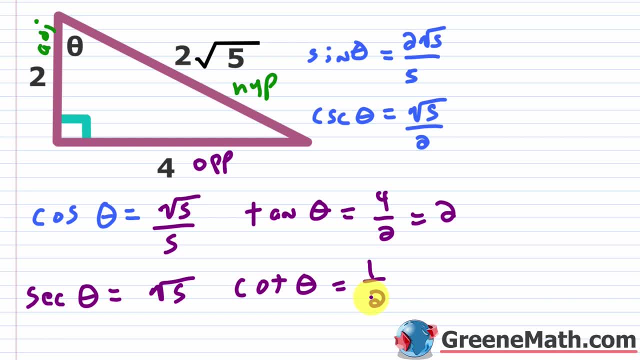 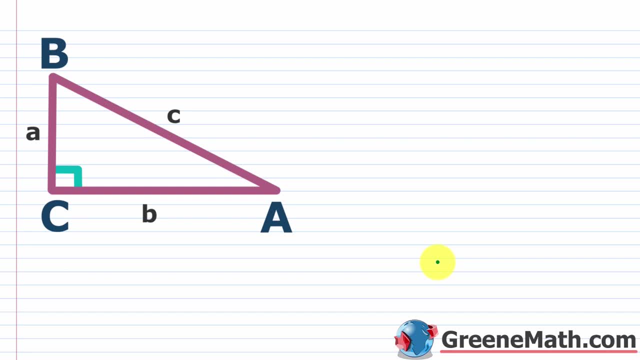 going to lead us to an important result, And we're going to talk now about something called co-functions. So to talk about these co-function identities, at least the first time you see them, it can be a little bit challenging to understand. So just stay with me for a moment. I'm going to 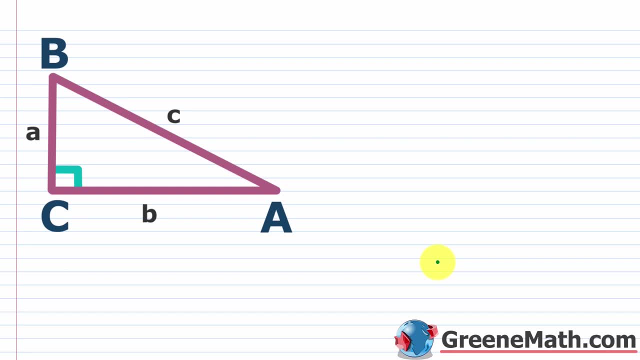 examples. They're very, very easy to figure out. Okay, So even if you don't fully understand the concept, you can work the problems very, very easily. So the first thing is that we noticed that the sine of theta from the first example was equal to the cosine of theta from the second. 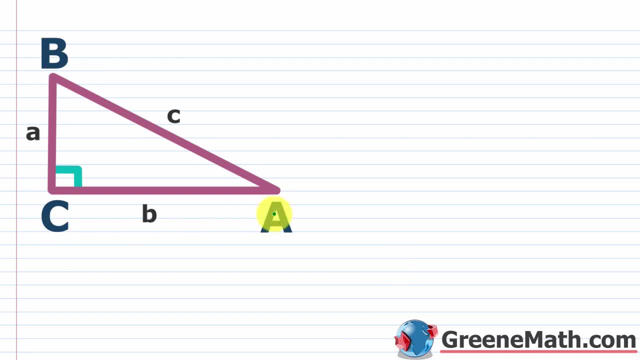 example. So I have the same triangle here, I've just marked it with different letters. There's no actual numbers here. Okay, So we have this lowercase a, this lowercase b and the lowercase c, that's representing the lengths of the sides here. Okay, So if we want to, 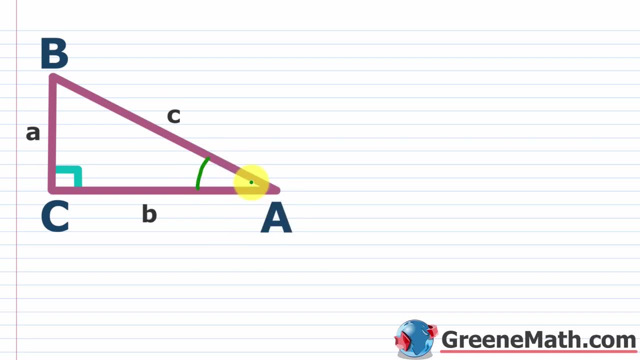 let's say, we had this measure of angle a, So this is angle a. This is what we used in the first scenario. If we wanted sine of a here, Okay, If we wanted sine of a, well, what is this going to be? 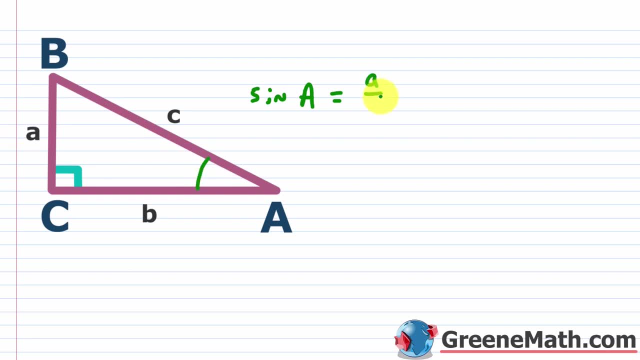 Well, it's opposite over hypotenuse. Your opposite here is the lowercase a, Your hypotenuse here is lowercase c. Okay, And then if you wanted the cosine, okay of b. now, okay of b, So I'm. 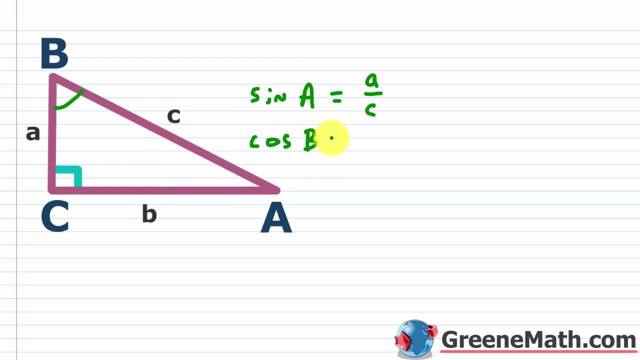 changing the angle up on here. now You're going to notice that's going to be the same thing. It's a over c And again, lowercase a, lowercase c, Because now this is your adjacent Okay, And this is still your hypotenuse. Remember, cosine is adjacent over hypotenuse And you'll notice that. 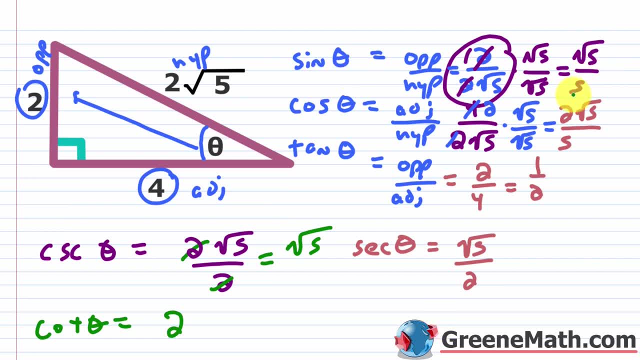 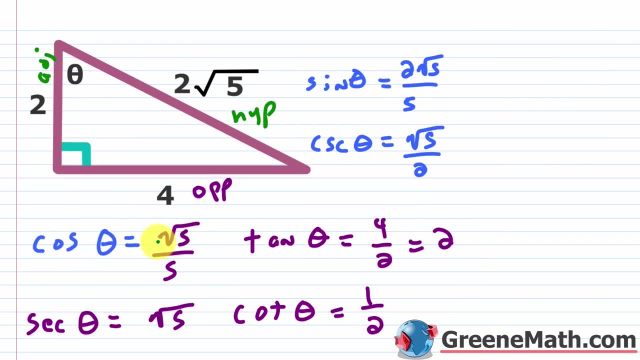 again, your sine of theta is the square root of five over five. This is the first example where this is our angle. In the second example, the cosine of theta- here's our angle- here- is square root of five over five. So this relationship is always going to be true for the two acute angles. 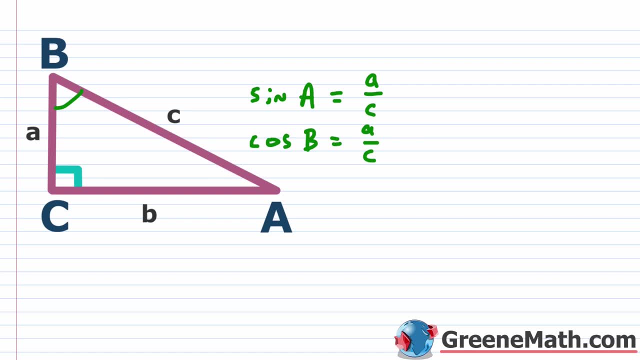 since the sum of the three angles in any triangle is 180 degrees And our angle c here- remember this, is our right angle- It's exactly 90 degrees. So that means, because the sum of all three angles is 180 degrees, the sum of the measures of angles b and a is going to be 90 degrees. right These. 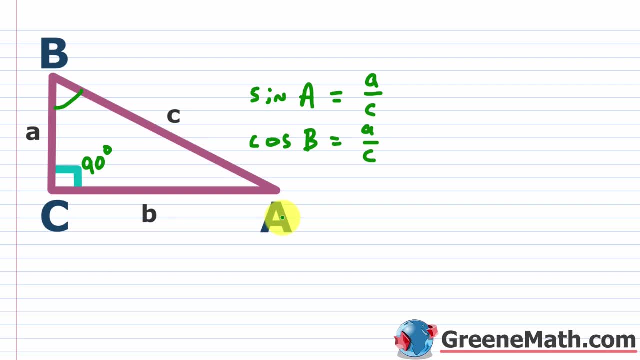 are complementary angles. We've talked about this before. If they sum to 90 degrees two angles, they're complementary angles. So because these two angles, a and b, are complementary, sine of a is equal to our cosine of b. We say the functions sine and cosine are co-functions. 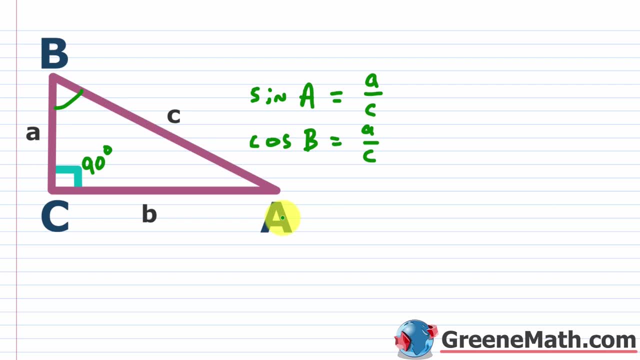 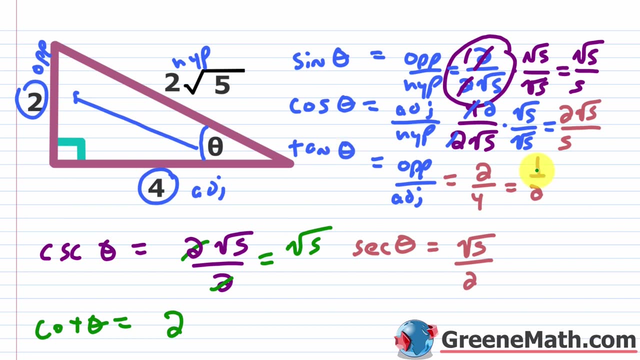 We also say that tangent and cotangent are co-functions, And then we can say secant and cosecant are co-functions as well. And if you want to go back, if you look at the tangent of theta here, it's a half. And if you look at the cotangent of theta here it's a half. Okay, If you look at 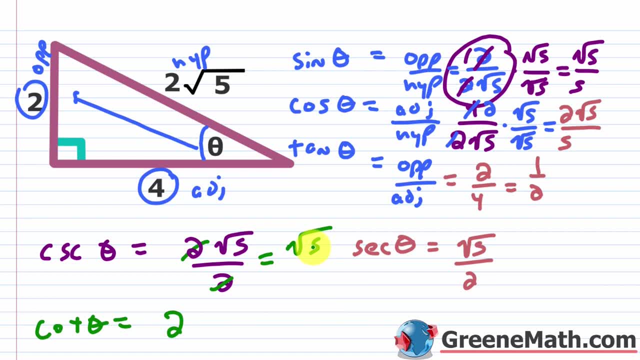 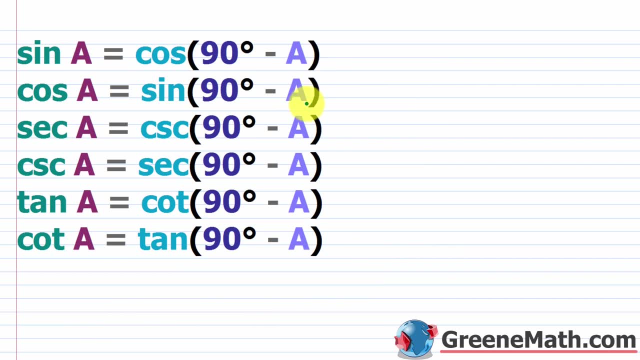 the cosecant of theta here it's square root of five. And if you look at the secant of theta here, it's square root of five. So how can we use this for practice problems? These are your co-function identities. You just 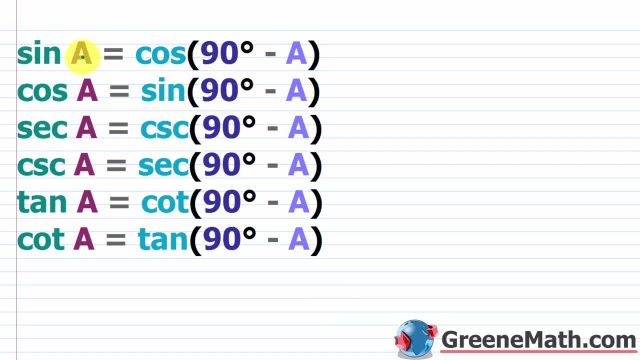 need to memorize them. It's something you're just going to plug into. So your sine of your angle a is equal to your cosine of 90 degrees minus your angle a. So, for example, if it was sine of 50 degrees, well, you would just say this is equal to cosine of. let me make this a little bit better. 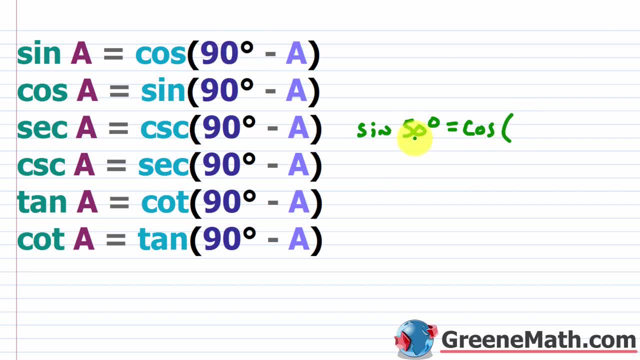 So cosine of what? Well, you would say 90 degrees minus 50 degrees, that's 40 degrees. Okay, And you can punch this up on a calculator and you see that those are the cosine of 90 degrees minus 50 degrees. 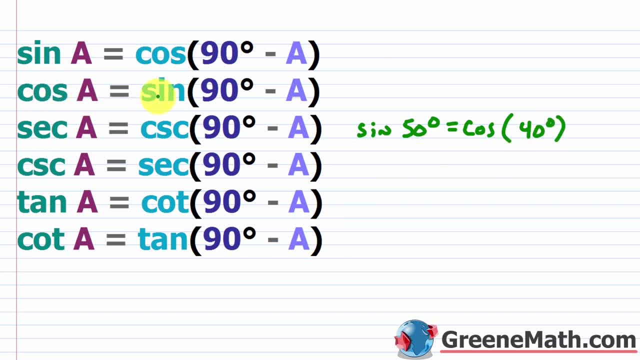 Okay, And you can punch this up on a calculator and you see that those are the same Same deal with cosine of a and sine of 90 degrees minus a, secant of a and cosecant of 90 degrees minus a, so on, and 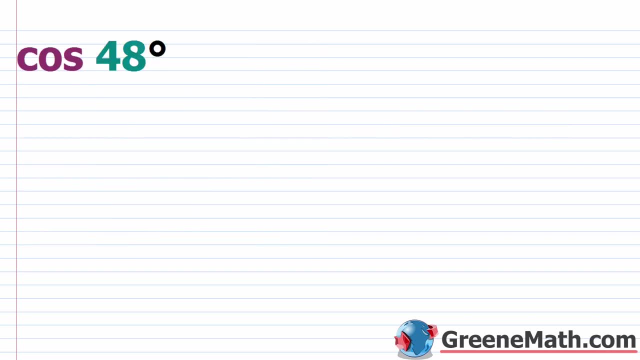 so forth. You can copy these down. But basically, if we look at a problem like this, the cosine of 48 degrees, and we want to write it in terms of its co-function, well, again, you just say well. 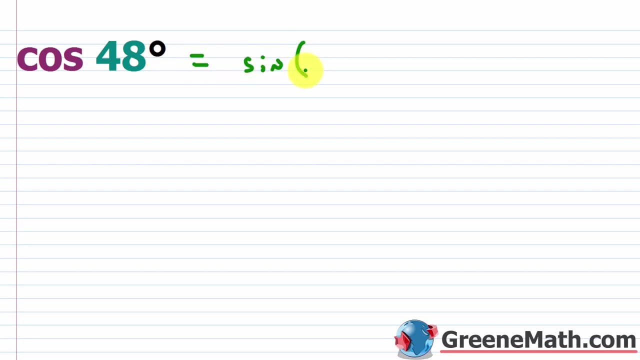 this is going to be equal to the sine of you take 90 degrees, 90 degrees minus the measure here, which is 48 degrees Okay. And what's? 90 degrees minus 48 degrees? Well, it's going to be 42 degrees Okay, So we can. 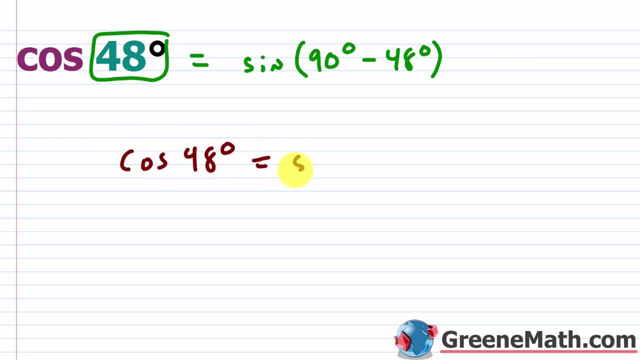 say, cosine of 48 degrees is equal to sine of 42 degrees. Okay, So this number here and this number here, those guys, because these are again complementary angles, they have to add up to 90 degrees. So that's what you want to make sure of, And then make sure your co-function is there. So 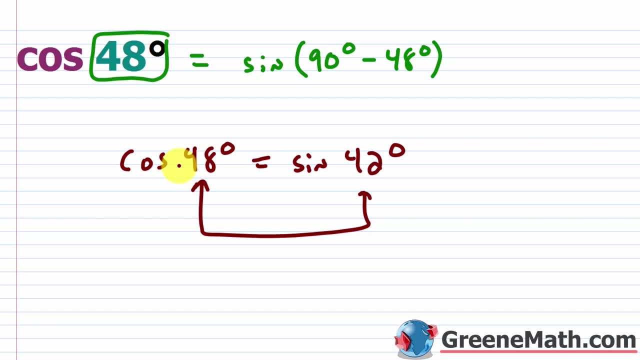 cosine and sine tangent and cosine secant and cosecant, so on and so forth. Let's do another, So we have the tangent of 11 degrees. So again, I would do co-tangent, okay, of 90 degrees minus 11. 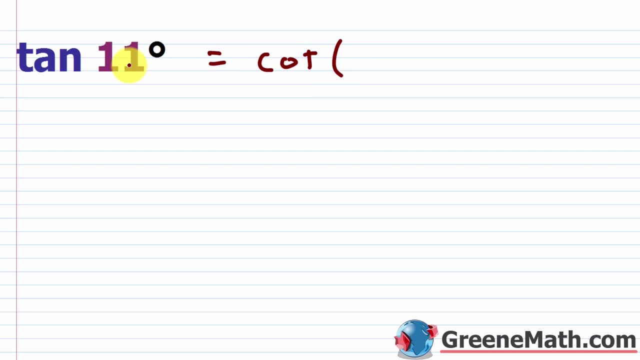 degrees. 90 minus 11 is going to be 79. So this would be co-tangent, okay, of 79 degrees there. So the tangent of 11 degrees is equal to the co-tangent of 79 degrees. Again, you want to. 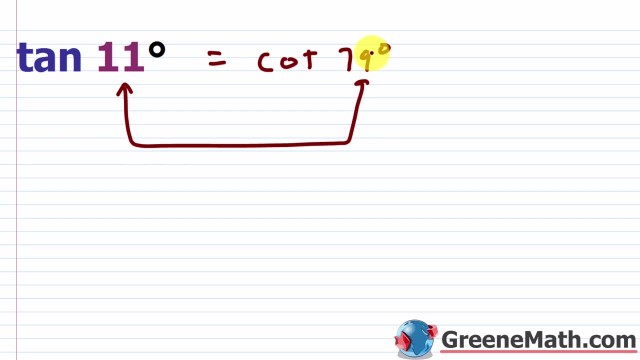 check to make sure that this plus this is going to give you 90 degrees, Okay. So let's look at an example that involves solving equations using co-function Identities. for this guy right here, we're going to find one solution for the equation, Okay, And 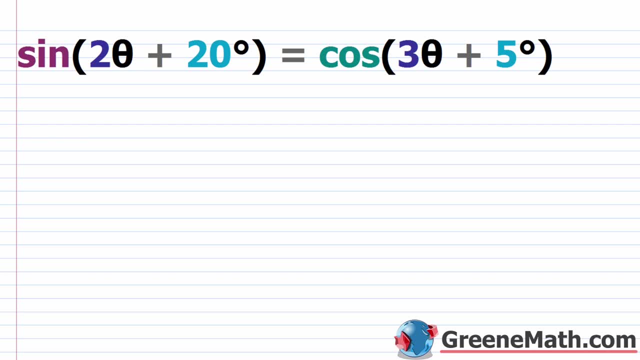 we're going to assume all the angles involved are acute angles. So you'll see a problem like this or a few problems like this in this section, and solving it is very easy. Remember I told you that this plus this, okay, is going to equal 90 degrees. So all I need to do is take the inside. 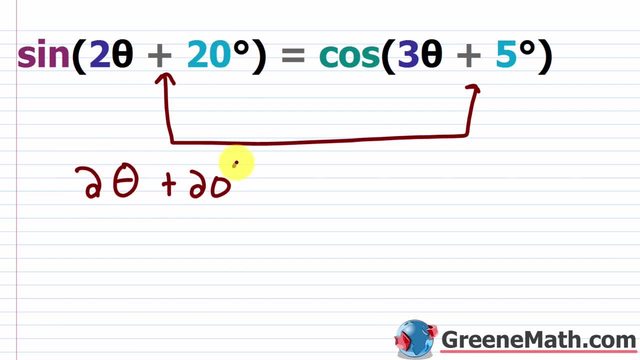 parts the two times theta plus 20 degrees and add this to the three times theta plus five degrees, And set this equal to 90 degrees. Okay, I'm going to solve for theta. okay, my unknown angle measure. So what I'm going to do here is I'm going to combine like terms, So 20 degrees plus five. 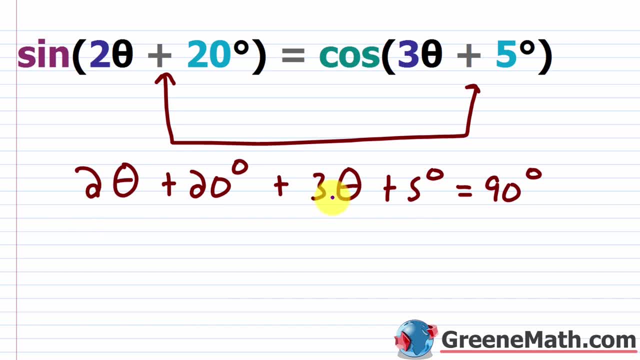 degrees is 25 degrees, And two times theta plus three times theta would be five times theta. So five times theta plus 25 degrees is equal to 90 degrees. Okay, So just like I'm solving an equation, just like if I had x there, I want to isolate this guy. So I want this by itself. 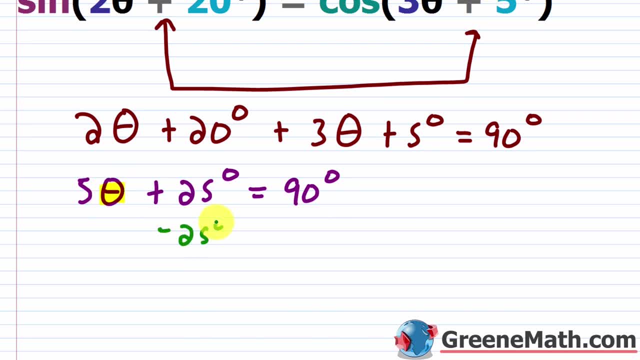 So how do I do this? I'm going to do this by isolating this guy. So I'm going to isolate this guy. I'm going to first subtract 25 degrees away from each side of the equation. So this is going to be. 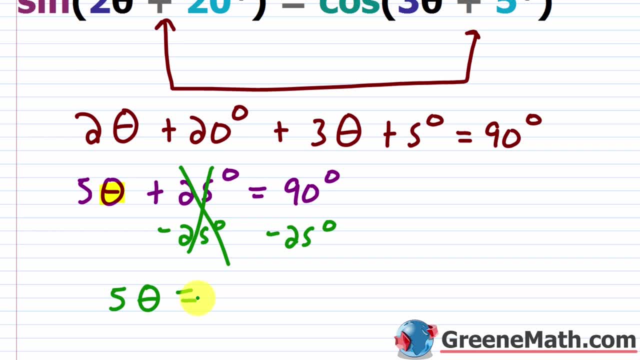 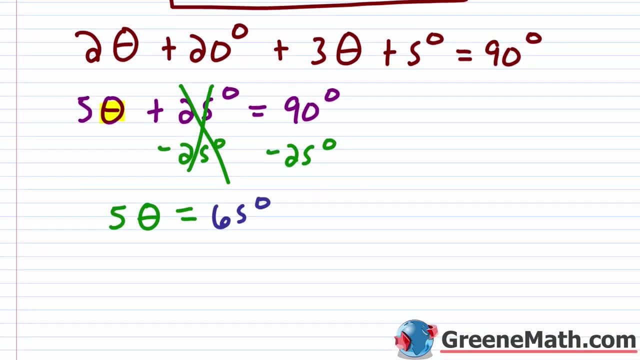 gone, I'll have five times. theta is equal to what's 90 degrees minus 25 degrees, It's going to be 65 degrees. Okay, So to wrap this up, what I'm going to do is divide both sides by five. 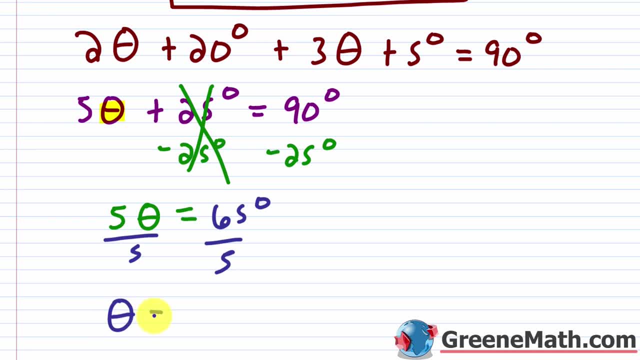 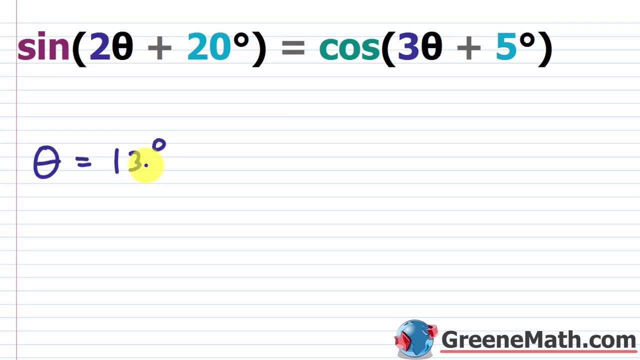 so that I can isolate theta. And I'll say that theta is equal to 65 divided by five is 13. And of course you have degrees there for the units. So I would say theta is equal to 13 degrees. Now, if you want to check this, all you would do is plug in. So two times 13 degrees is 26 degrees. 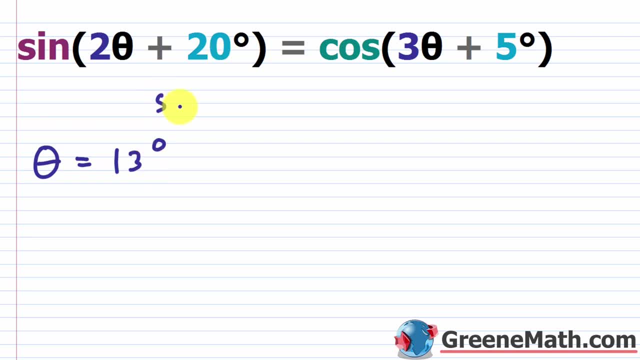 26 degrees plus 20 degrees is 46 degrees. So sine of 46 degrees is equal to cosine of what. Three times 13 degrees is 39 degrees. 39 degrees plus five degrees is 44 degrees. So is this true? Yes, it is right. Sine of 46 degrees is equal to cosine of 44 degrees. Again, 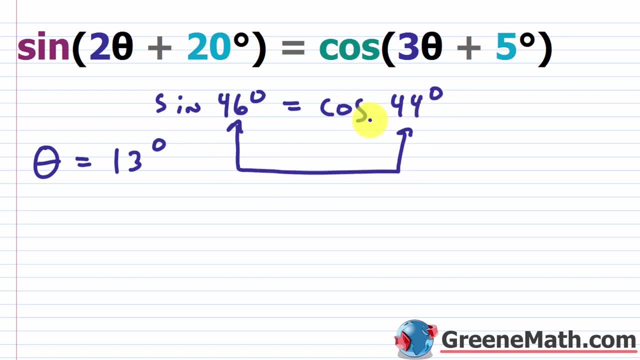 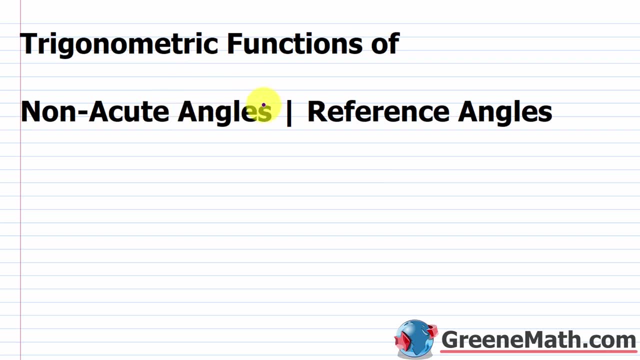 this, plus this has got to be 90 degrees And of course, you have your sine and cosine. In this lesson, we want to talk about trigonometric functions of non-acute angles, and also we'll learn about reference angles. All right, So let's start off with a concept. 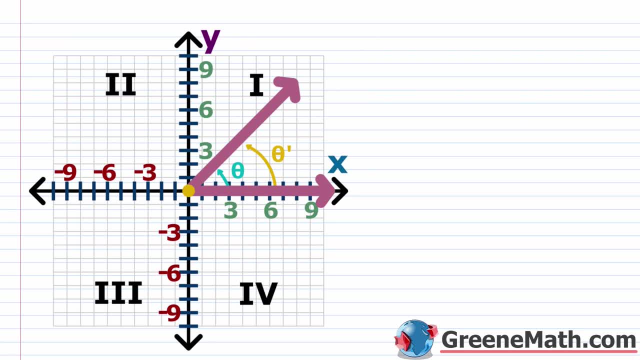 of a reference angle. This is something that's very important in trigonometry. So first, from the definition, we're going to say that every non-quadrantal angle, in standard position, will have a positive acute angle known as its reference angle. So when we talk about the 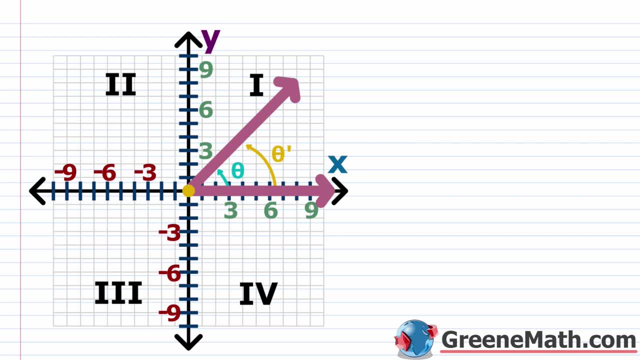 reference angle for an angle theta. it's written as theta prime, So you'll see, here we have this theta prime. Okay, So this is your reference angle notation. Now, when we talk about the reference angle for an angle theta, then basically this is the positive acute angle that is made by the. 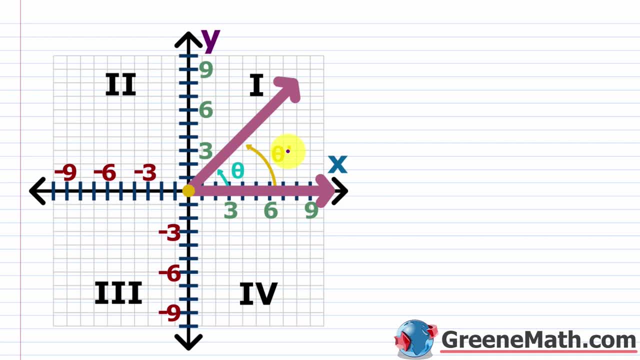 terminal side of our angle theta and the X axis. So I'm going to go through this in each quadrant. In every case, I'm going to be thinking about an angle theta that is between zero degrees and 360 degrees. If you get something that's outside of the angle theta, then you're going to be thinking about. 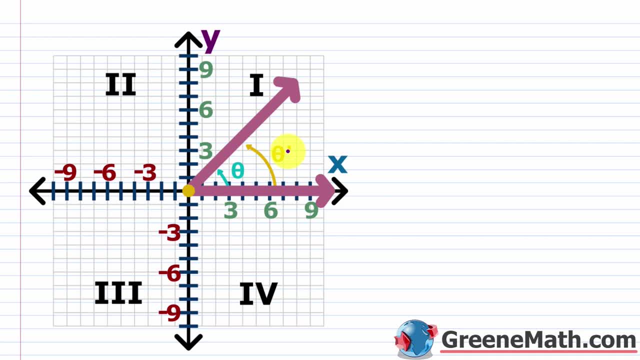 that You're just going to find the coterminal angle, that's between zero degrees and 360 degrees, and you'll apply the little formulas that we're going to look at here. So what I'm going to start with is an angle in quadrant one. So if I think about the positive acute angle that is made from, 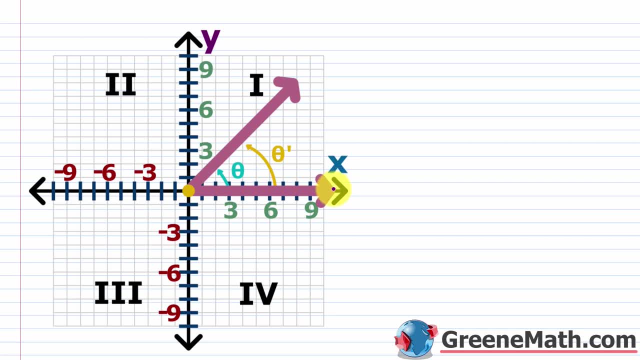 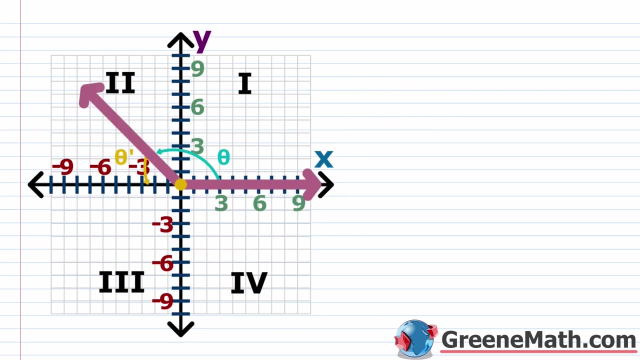 the terminal side of this angle, theta, and the X axis. well, easily I can see that theta here is going to exactly be equal to theta prime. So if you're in quadrant one then you can say that angle theta is going to be its own reference angle. If you're in quadrant two, you have to do: 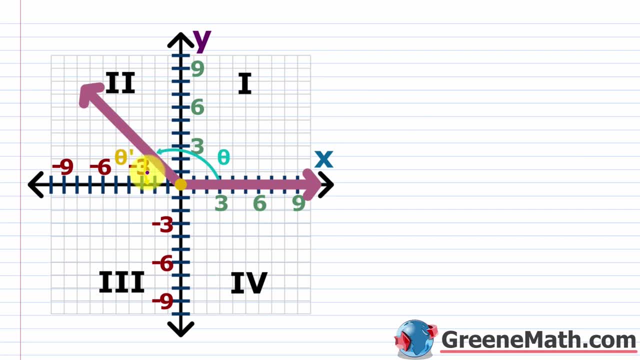 a little bit more thinking. So now I'm thinking about this angle right here. Okay, so this is my theta prime. Let me use a different color that's going to show up here. So this is from the terminal side of this angle, theta to the X axis. So I'm always thinking about going to the 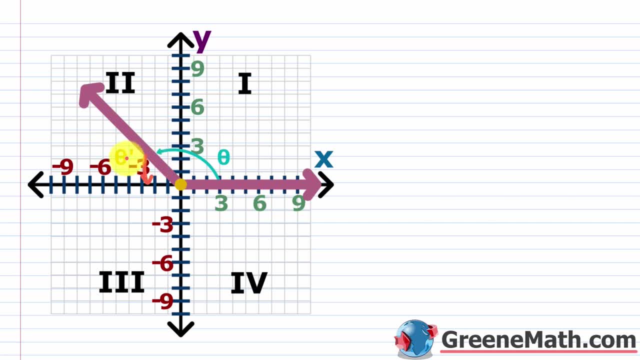 X axis, So that angle has this measure of theta prime. So how do we get this? What I would think about is the fact that if I took this angle measure here, which is a straight angle, the measure is 180 degrees. So I'm going to say in quadrant two, I'm going to start with that. 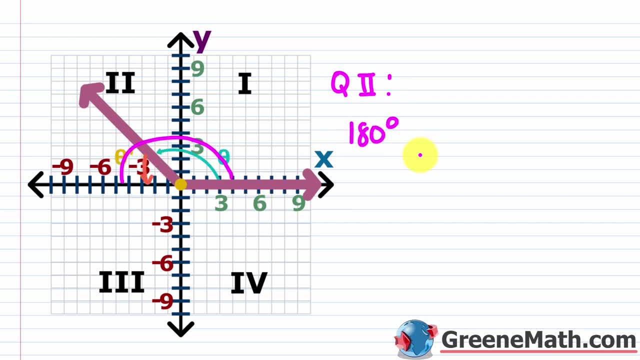 straight angle, which is 180 degrees, And I'm going to say that I need to subtract away the measure of the angle, theta, right? So I'm going to take this part away, right? That's what I'm going to subtract away And that's going to leave me with my theta prime that I'm looking for. Let. 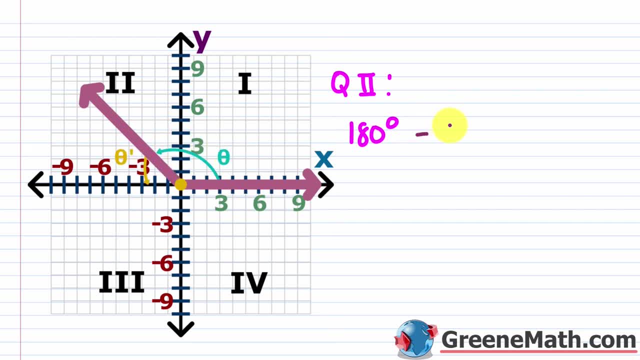 me get rid of all this. So that's more clear. So I'm going to subtract away my angle, theta, whatever it is, And let me slide this down here And I'll say that theta prime, or your reference angle, is going to be equal to 180 degrees minus. 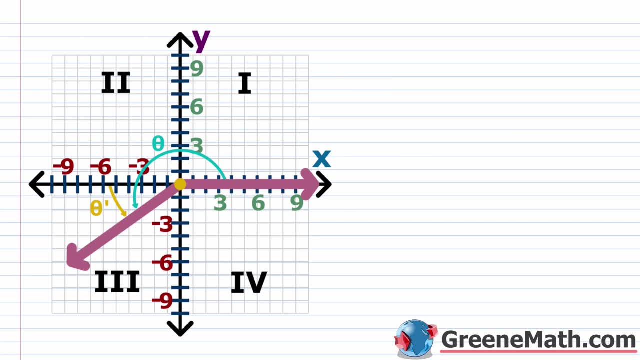 theta. Again, this is in quadrant two. All right if we're in quadrant three. well, now we have to think about this guy right here. So this is your angle here And I only want this part right here. So, coming from the X axis going down to that terminal side, that's going to be my theta prime. 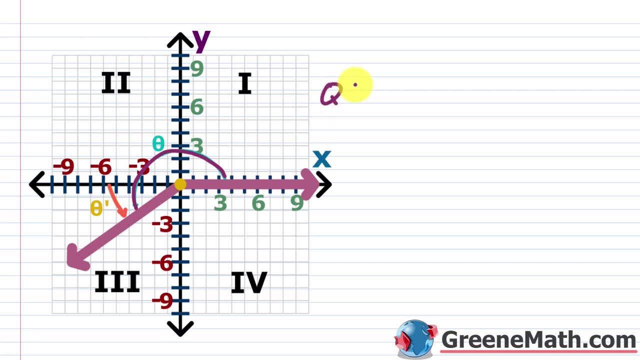 here. So in this particular case, in quadrant three, we are going to start with our angle theta. So let me say theta prime, That's equal to our angle theta, whatever it is, And we are going to subtract away this straight angle here. So this part right here, that's what we want to take out And that's going to leave us. 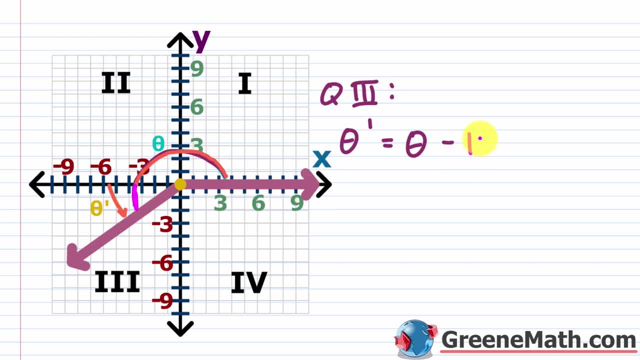 with this amount of rotation right there. So I'm going to take away that straight angle, which is 180 degrees. So in quadrant three, your theta prime, or your reference angle, is your theta minus your 180 degrees. All right, now let's take a look at an angle that's going to be in quadrant four. 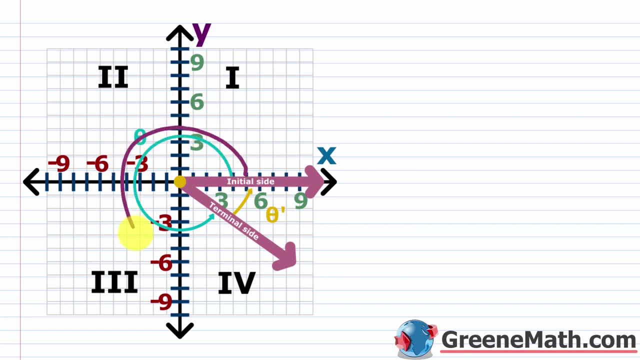 So if we think about one full rotation, so this guy right here, this is going to be 360 degrees. So if I'm in quadrant four, I would start with 360 degrees And then to get this angle, theta prime here, which is going to be this part right there. Well, all I 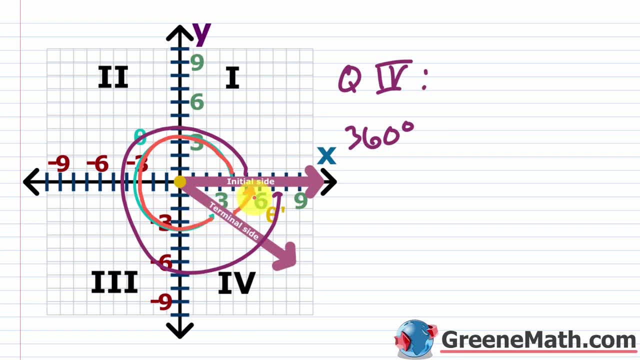 need to do is subtract out this angle here, theta right. I'll be left with my theta prime, So let me actually slide this down just a little bit And I'll say that theta prime is equal to 360 degrees minus my angle theta. Okay, so we have summarized everything. 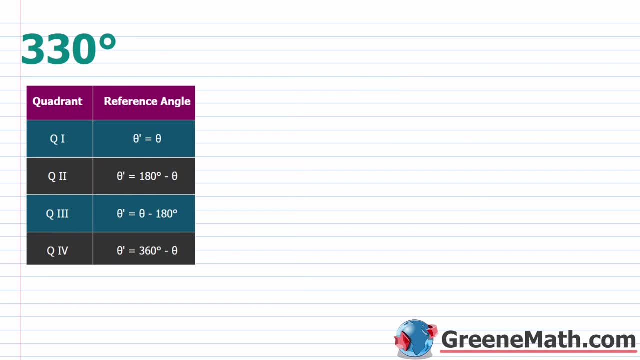 And basically, when you get to the examples, once you've gone through how it works, you can just use this little table After you work enough examples of this or get deeper into trigonometry. this is something you're just going to have memorized And you won't have to consult a. 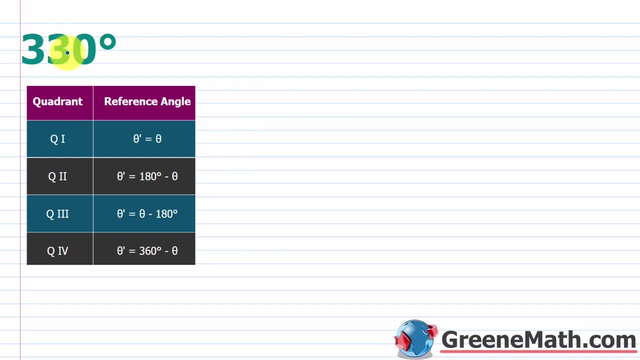 table or draw a sketch or anything like that. So I'm going to start out with 330 degrees And I want to find the reference angle. So I know that this is in quadrant four. So I look through my little cheat sheet here And in quadrant four again, my theta prime is going to be 360 degrees. 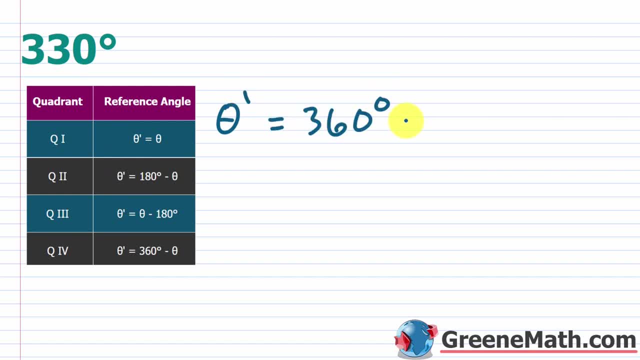 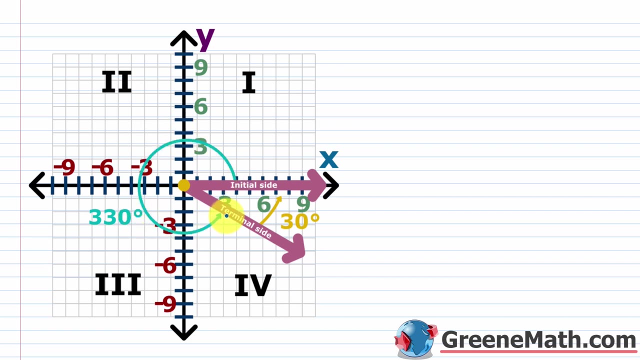 theta prime is equal to 360 degrees minus my angle theta. in this case it's 330 degrees, And so this is just going to be 30 degrees for the reference angle, And again, you can always make a sketch if this is not clear for you. So this would be a 330 degree angle And a lot of you can. 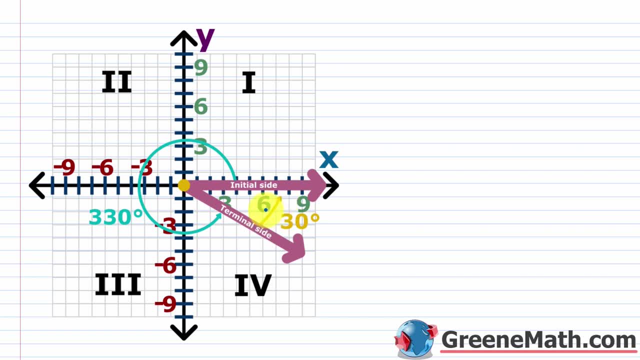 just think about that and see that I would need 30 more degrees to get back to the x axis. So that's your reference angle there. But again, you can also do it where you think about one complete rotation is going to be 360 degrees, so 360 degrees, and then you subtract away the part that you're not. 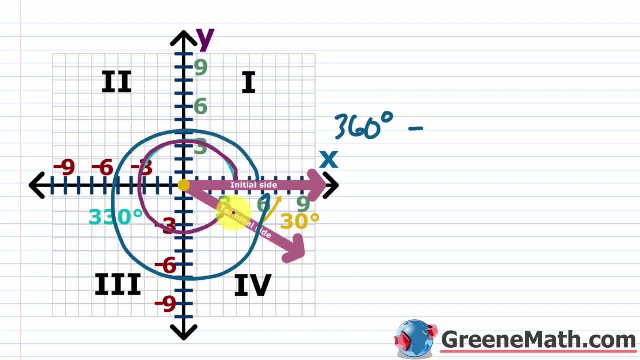 going to want to measure. So that's your angle, theta there, And in this case, that's your 330 degrees, And that leaves you with your reference angle, which is this part right here, which is 30 degrees, right? So let me put theta: prime is equal to this. okay, for the next one, we have negative. 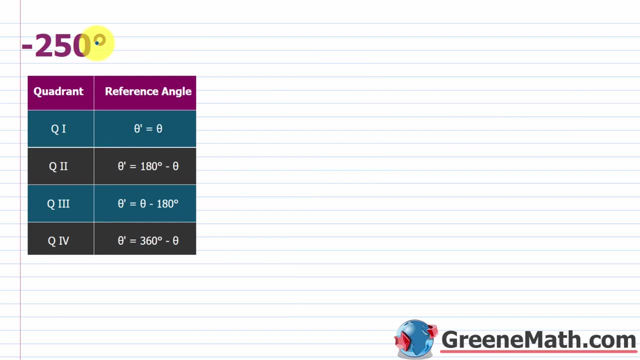 250 degrees. So, as I mentioned earlier, if you're not between zero degrees and 360 degrees, find the coterminal angle Now. you could do it this way, And a lot of people do, But I think finding the coterminal angle first is just worthwhile, because it's just going to make 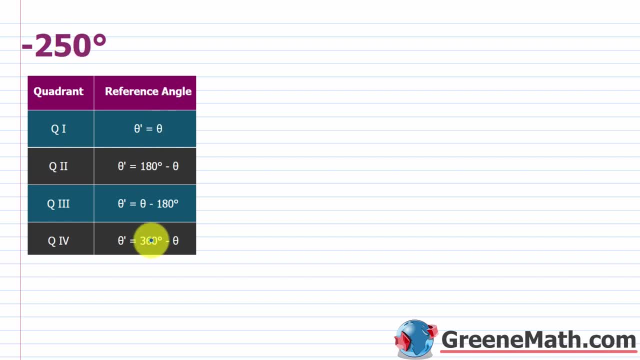 the process easier. you can just use this. So for negative 250 degrees, I would start by just adding 360 degrees to find my coterminal angle, And that's going to give me 110 degrees. So now I'm thinking about a theta of 110 degrees. that's going to be in quadrant two, So in quadrant two. 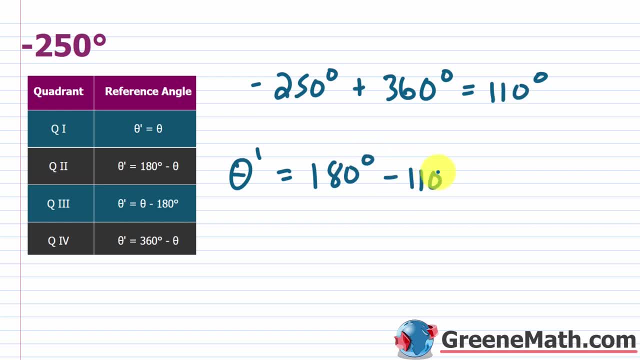 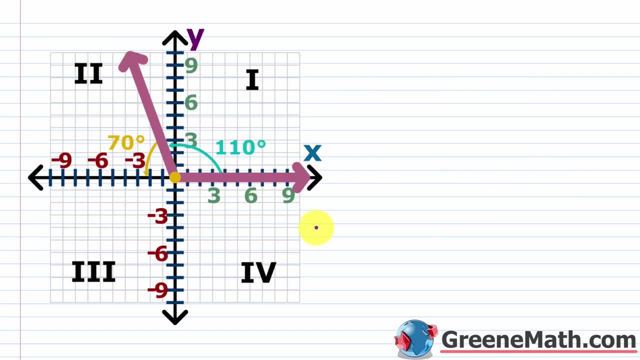 180 degrees minus this 110 degrees, and that's going to give me 70 degrees. So again, if you want to look at a little sketch, we think about an angle with a measure of negative 250 degrees. we're going to show that with a clockwise rotation. So I'm going to start here and go. 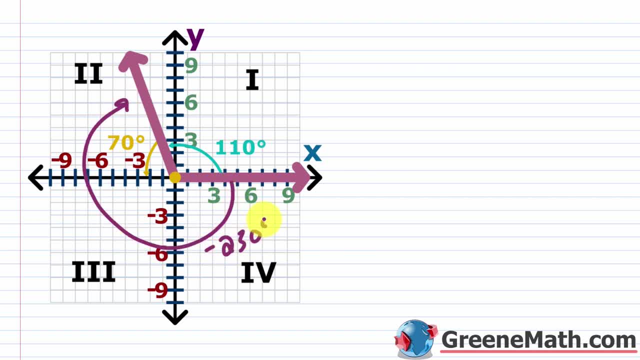 this way. So that guy would be negative 250 degrees, But again you just work with the coterminal angle, right. So that's 110 degree angle, same initial side, same terminal side. And so let's get rid of this And we'll just 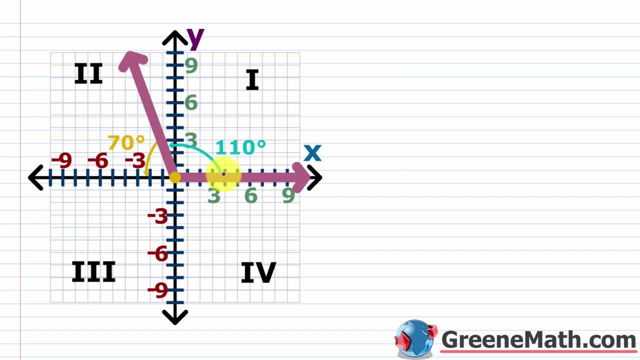 work with this guy. And again, you can think about this logically: if I start here and I rotate 110 degrees counterclockwise, well then I need to go another 70 degrees to get to the x axis. right. 110 degrees plus 70 degrees is going to be 180 degrees or form that straight angle. 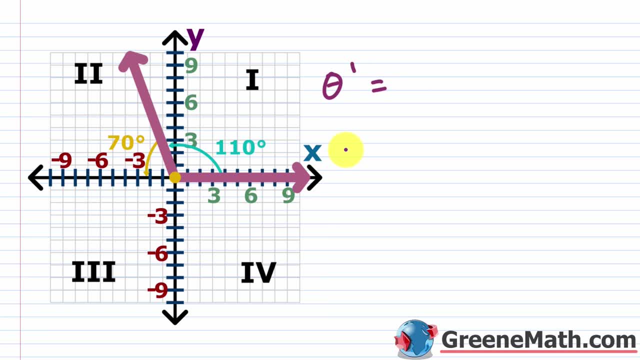 Again, the other way you could think about it is: your theta prime here is going to be your straight angle, which is 180 degrees, minus the part of this rotation that you don't want. So that's this part right here, which is your 110 degrees. So that's going to be your theta prime here. 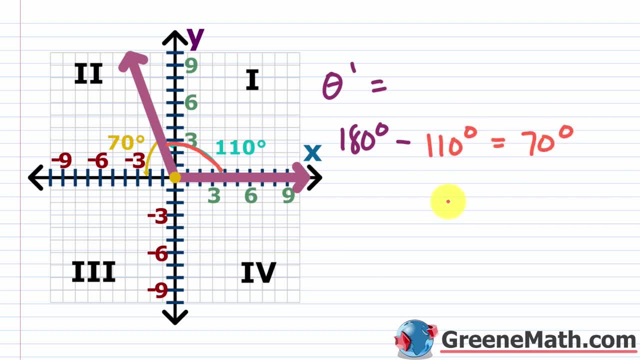 angle, And so that's 70 degrees. Okay, so that's your theta prime or your reference angle. All right, let's look at one more. So now we have 560 degrees, And again I would find the coterminal. 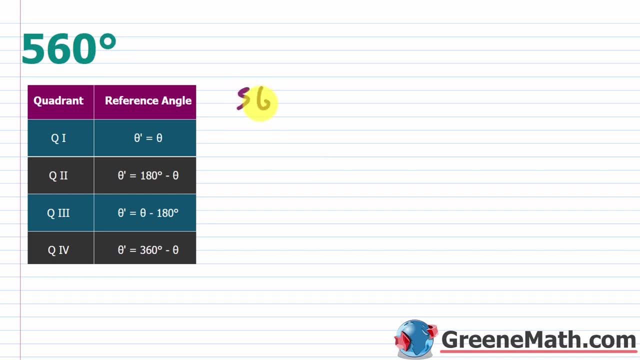 angle that's between zero degrees and 360 degrees. So 560 degrees, let's say minus 360 degrees, And that's going to give me exactly 200 degrees. So this angle right here is going to be in quadrant three. So in quadrant three we would say theta prime is going to be theta, which is 200 degrees. 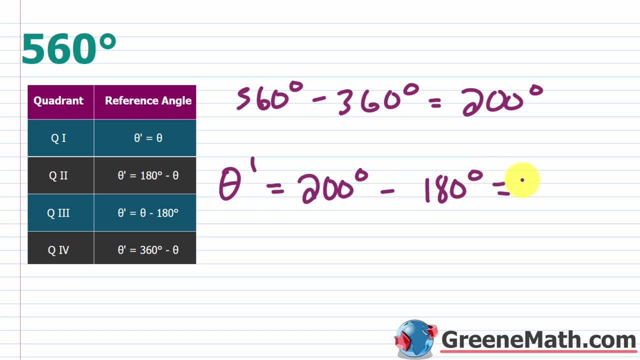 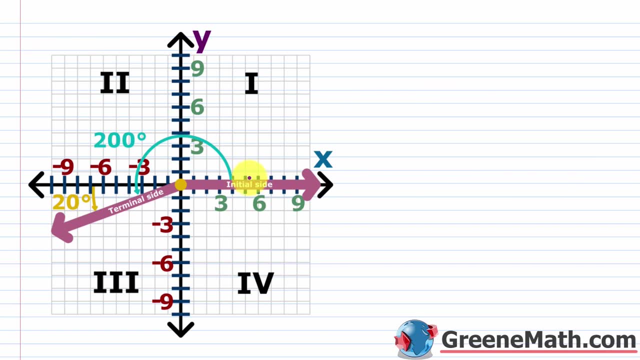 minus 180 degrees. So my reference angle, theta prime, is 20 degrees. So, coming to our little sketch again, if you wanted to think about it as a 560 degree angle, that's one complete rotation which is 360 degrees and then another 200 degrees to get to that point right there. But I just like 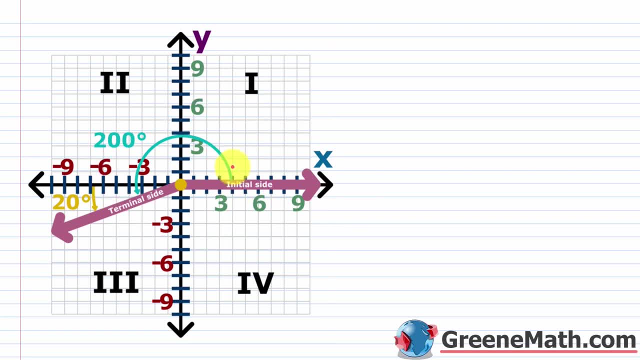 to work with the coterminal angle. I think it's much easier In this particular case. you think about the entire rotation here. So let me put theta prime is equal to, that's going to be 200 degrees, And then you want to subtract out the part that you don't want. Again, I'm thinking about from. 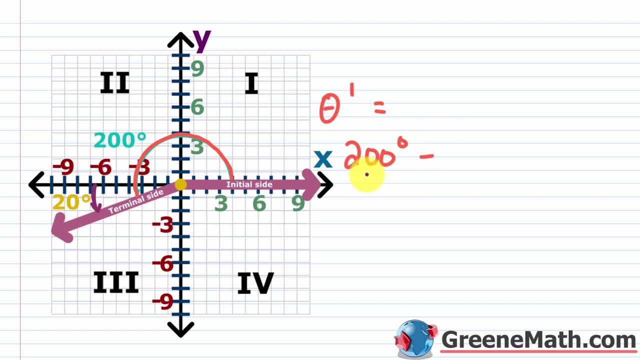 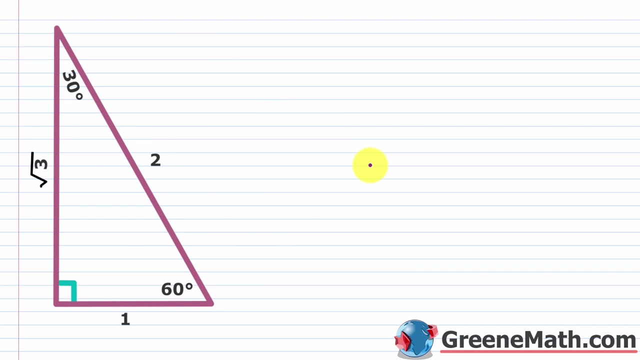 here, the x axis to here. So that's going to be me taking out this straight angle here, which is going to be 180 degrees. So that gives me my reference angle, or this rotation from here to here of 20 degrees. Alright, so now what we're going to do is talk about trigonometric function values. 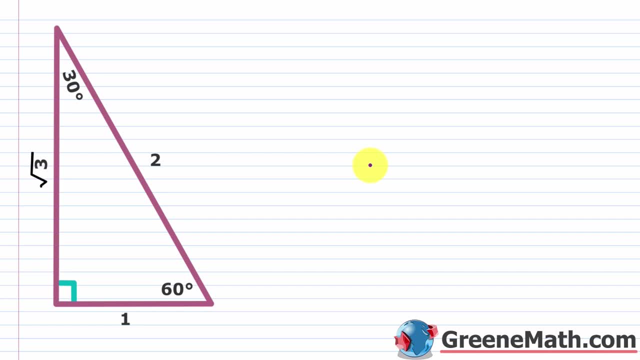 of special angles. So we have these 30 degrees, 45 degrees and 60 degrees in terms of the angles that we want to write. So a 90 degree angle, let's say, is the 30 degree angle we're looking for is. 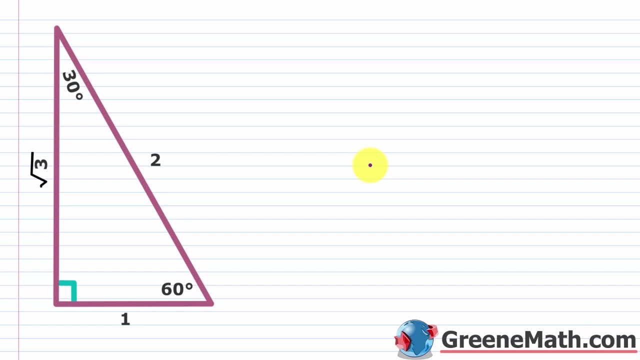 the side that's opposite of the 30 degree angle has the exact length of one. the side that is adjacent to this line right is the side that is adjacent to this line. Now. now let's talk about the side that is opposite of the 30 degree angle, because we want to learn about that And we want 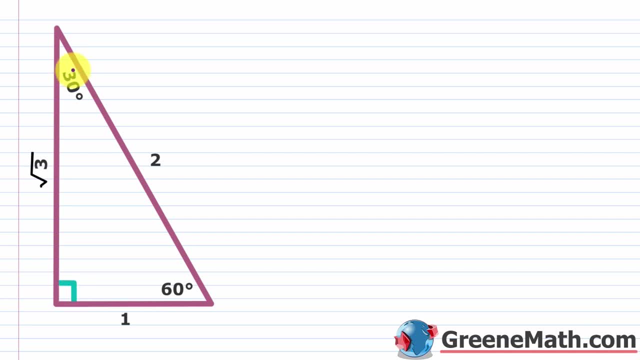 to memorize the sine, cosine and tangent values for, and then also your reciprocal functions. So your cost secret, your second and your cotangent. So I'm going to start off with a triangle that you should know from geometry if you haven't taken geometry before. it's not that big of a deal. So this triangle, 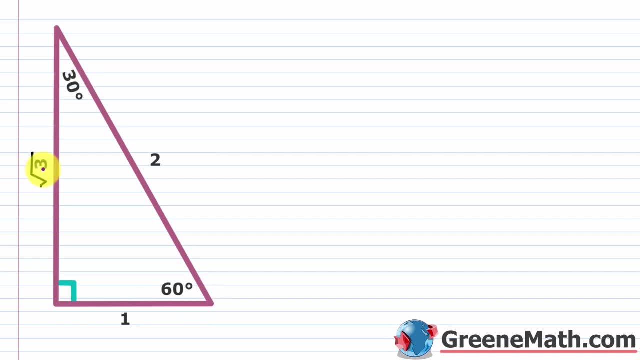 is known as a 30 degree, 60 degree, 90 degree triangle. So this is a special right triangle, And so the side that's that is adjacent to this 30 degree angle has length squared of three. And then the hypotenuse. 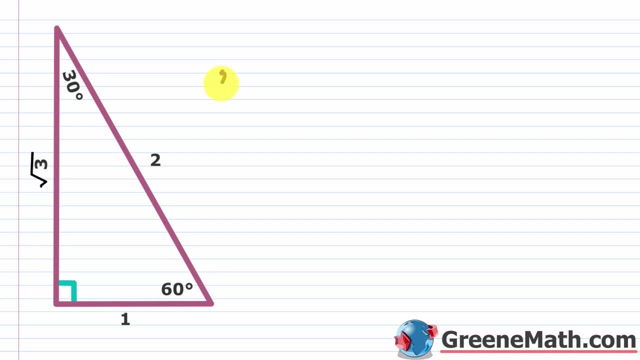 here has length two. So if I wanted to figure out the sine of 30 degrees and then the cosine of 30 degrees and then the tangent of 30 degrees, let's go ahead and set those up. So for the sine of 30, 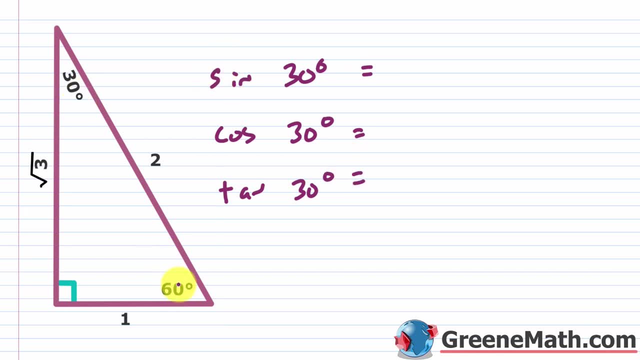 degrees. let me make this s a little bit better. Again, it's opposite over hypotenuse. So the opposite side here has length one and the hypotenuse has length two. So this is one half Then for the cosine of 30 degrees. it's going to be adjacent, which is square root of three. 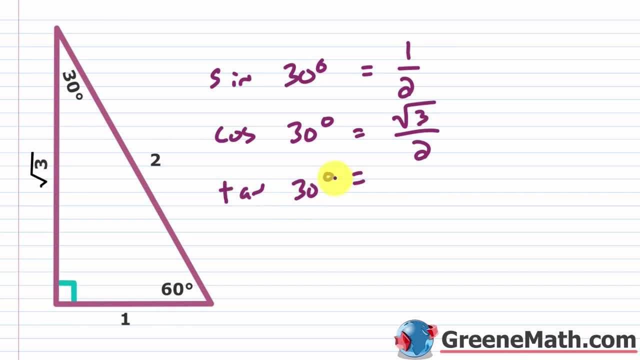 over hypotenuse, which is two. Now for the tangent of 30 degrees it's going to be opposite, which is one over your adjacent, which is square root of three. And of course we would rationalize the denominator there. So multiply by the square root of three over the square root of three. So 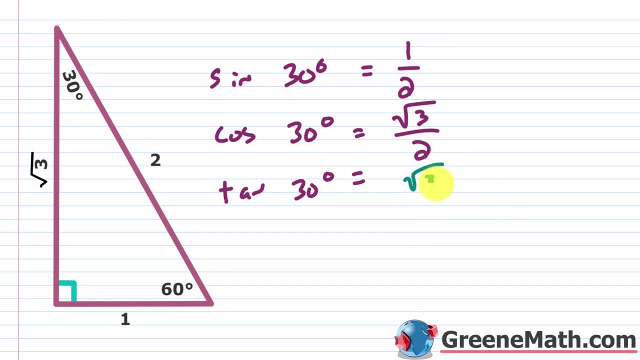 this is the square root of three over three. So square root of three over three. So square root of three over three. Now you could find your reciprocal functions if you wanted to. So you could take the reciprocal of this to get your cosecant of 30 degrees. you could take the. 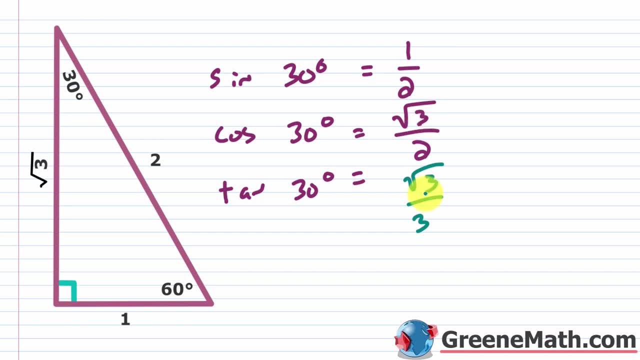 reciprocal of this to get your secant of 30 degrees, And you could take the reciprocal of this to get your cotangent of 30 degrees. I'm not going to waste time doing that. I'm going to give you a table where everything's presented, just showing you where this stuff is coming from. I'm going to 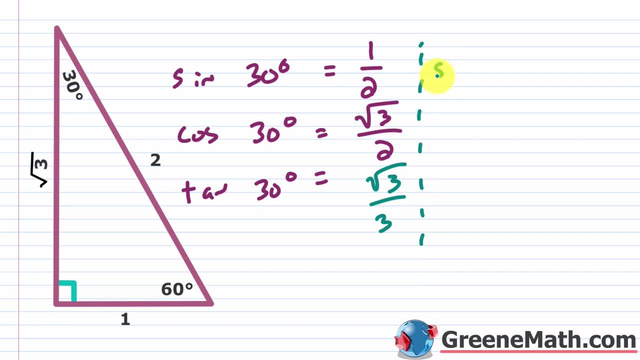 do the 60 degree angle as well. So let me go sine of 60 degrees, And we know from a previous lesson that that should be equal to the cosine of 30 degrees. So this should be the square root of three over two, And if we check that, well, if I look at the 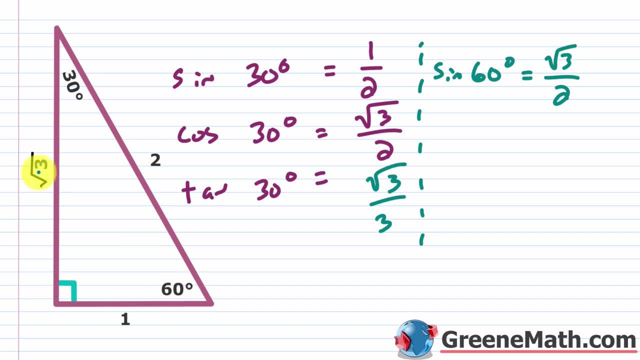 60 degree angle here. well, the opposite is now going to be the square root of three and hypotenuse is still two, so square root of three over two. So that checks out then the cosine of 60 degrees. again, we know that should be the sine of 30 degrees. So this should be one half. So if I 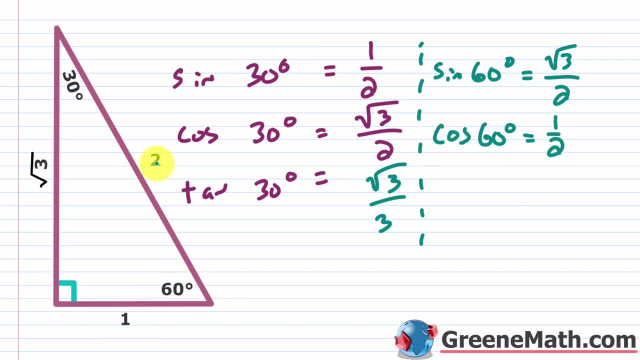 look at my cosine of 60 degrees. it's the adjacent, which is one, over the hypotenuse, which is two. so I do get one half then. for my tangent of 60 degrees, this is going to be equal to what? 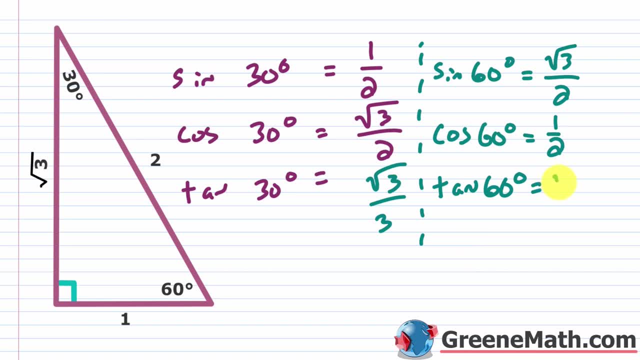 Well, again, I would just think about my opposite, which is square root of three over my adjacent, which is one. So square root of three over one is just going to be the square root of three. So the other angle that we didn't do was the 45 degree angle. So this is an isosceles triangle. 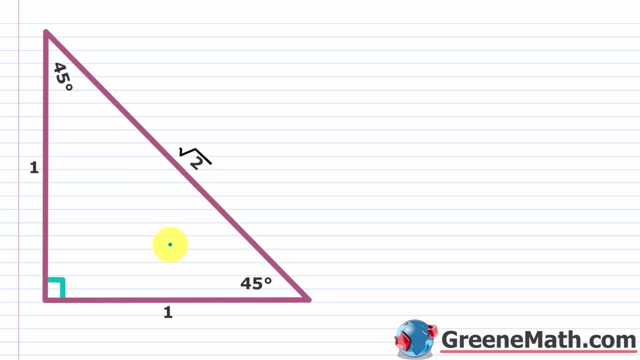 It's the 45 degree. 45 degree, 90 degree. That's a special right triangle from geometry. Again, if you've never seen this before, it's not that big of a deal. just showing you where the things come from. So if I want to write out the sine of 45 degrees, the cosine of 45 degrees and then the 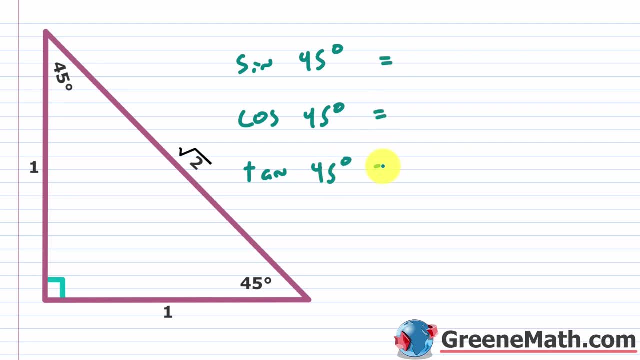 tangent of 45 degrees. So for these two it's going to be the same. Because, let's say, I start with this guy right here. Well, it's going to be the same as if I worked with this guy right here. doesn't matter, They're both 45 degree angles. So if I take this one right here and I say: 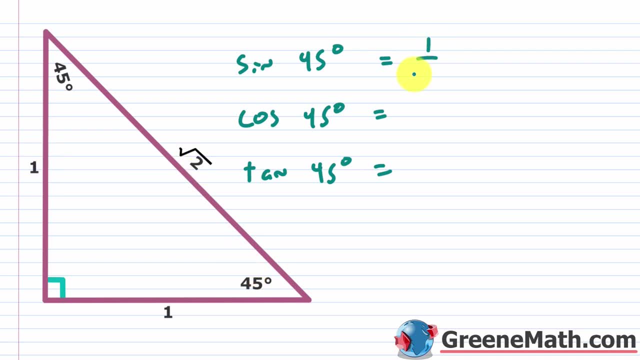 opposite over hypotenuse, it's going to be one over the square root of two And if I rationalize the denominator, multiplied by the square root of two over the square root of two, So this is the square root of two over two. So this is the square root of two over two. Now let's say- I start here- 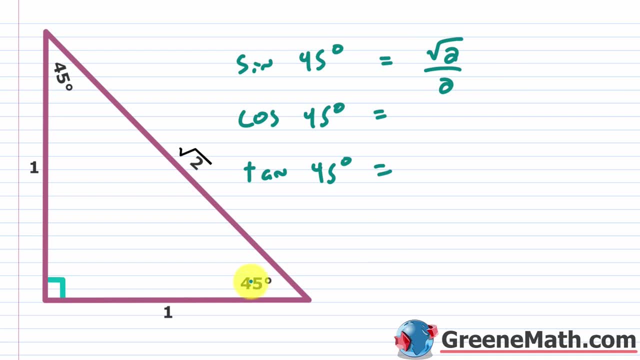 and I say: what's the cosine of 45 degrees? Well, now it's going to be adjacent, which is one over your hypotenuse, which is square root of two. Well, I just did that. So if I rationalize the 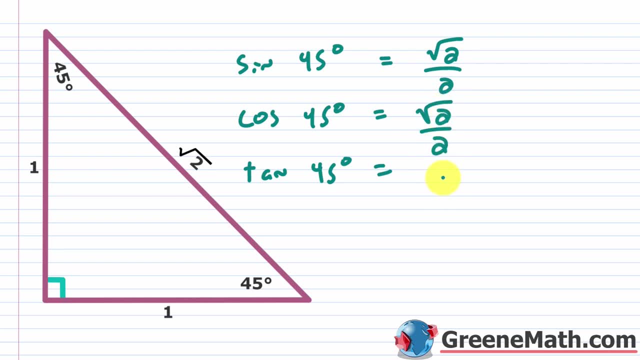 denominator, it's square root of two over two, And it wouldn't have mattered if I would have used this angle here. I would get the same result. Okay, now the tangent of 45 degrees. you're opposite, So let's use this one, So the opposite is one. and then over your adjacent, which is one. 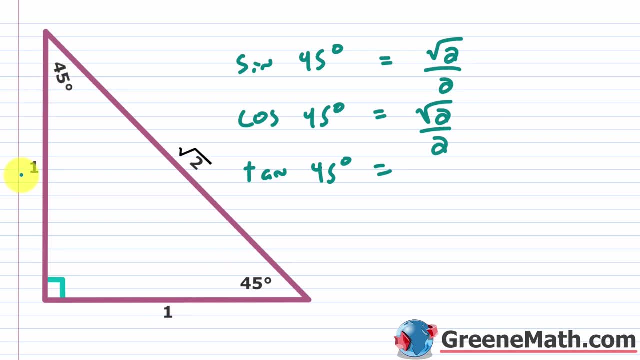 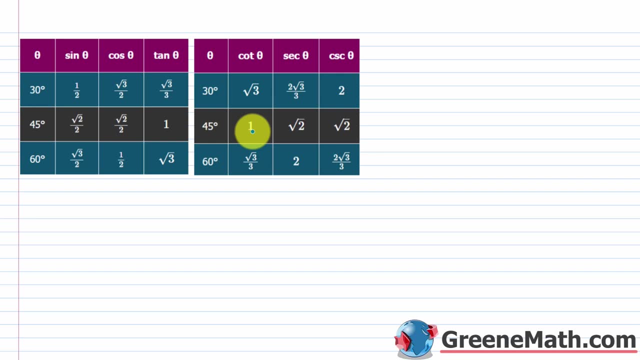 And again, if you pick this one, well, now the opposite is one and your adjacent is one, So it does not matter, It's one over one, which is one, Alright? so what I've done here is actually summarized all the information into a nice little table, So we already know where this information. 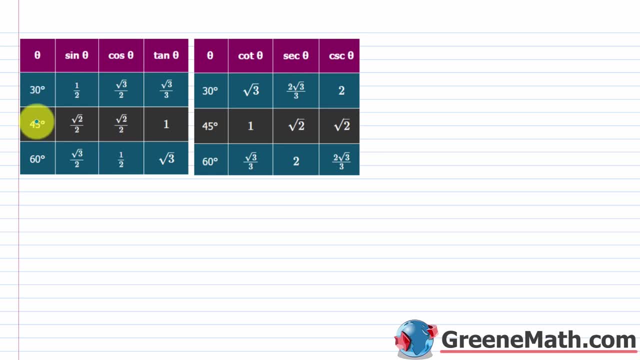 comes from. we looked at the sine cosine and tangent for 30 degrees, 45 degrees and 60 degrees. For this table over here, where we have the cotangent, the secant and the cosecant for 30 degrees, 45 degrees and 60. 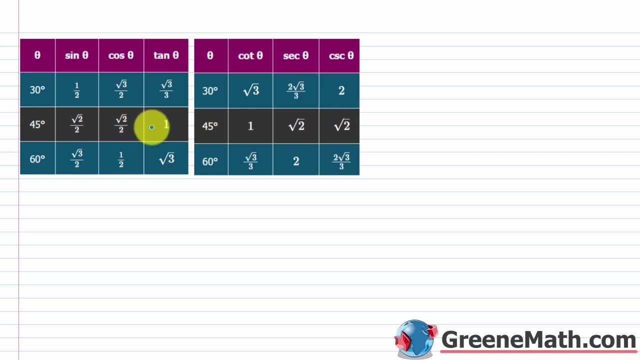 degrees. it's just found using the reciprocal identities. This is something you definitely want to commit to memory. these angles are going to come up over and, over and over again, So it's just going to make your life a lot easier. Now there's something you can search for called the. 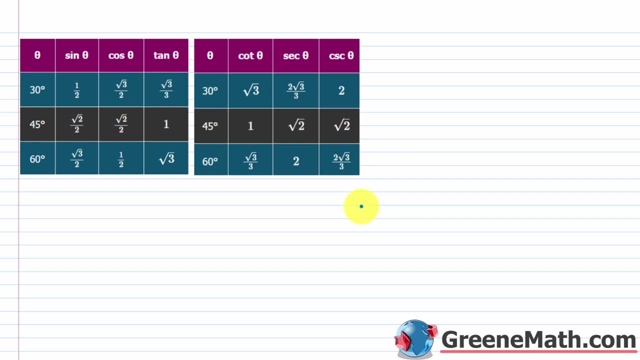 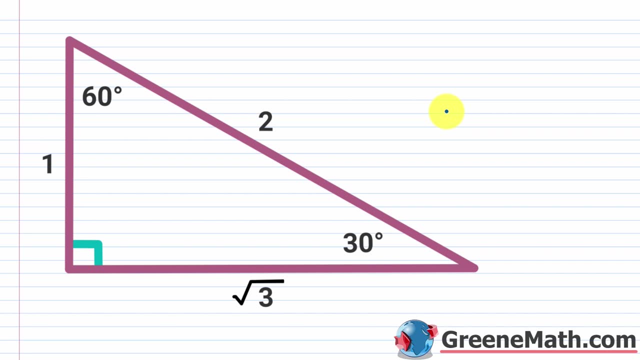 hand trick if you want an easy way of memorizing this. Alright, now let's talk about how to find the trigonometric function values when you have a non acute angle, but your reference angle is still going to be 30 degrees, 45 degrees or 60 degrees, So we're going to be able to use that. 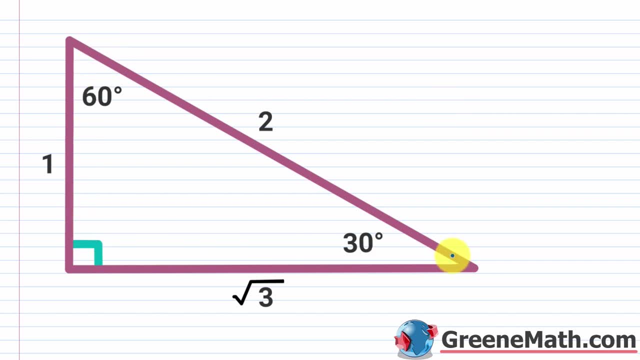 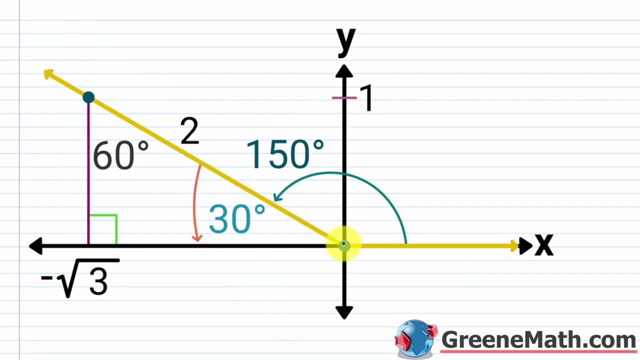 triangle and write a trigonometric equation. and then the point here: let's call our hand trick, Alright. so we actually don't really know where this is going to take us right now, but we have a whole lot here and we're going to do a little За and a Ra for that. then we're going to go ahead and 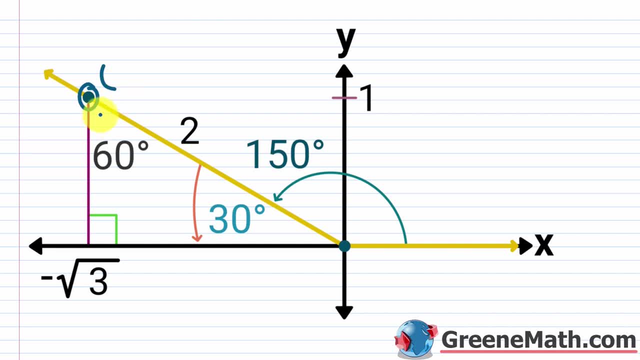 call it our table of coordinates. All right, let's quickly talk about how we're going to do this, because you'll see that we don't really have any Calledいう. we're going to find the x value and the y value, And we'll talk about that in a second, But again, 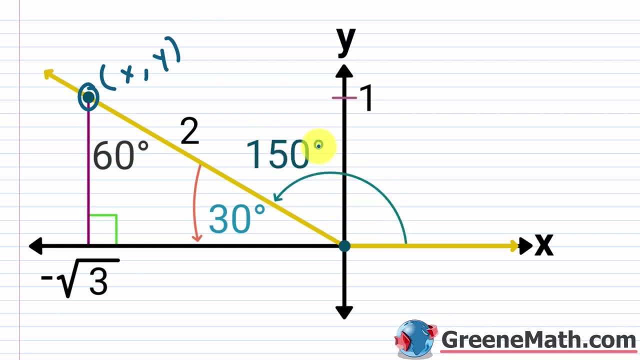 if you wanted to find the sine of this angle, which is 150 degrees, well, basically, you would just find that point on the terminal side And remember you have, sine of 150 degrees is equal to y over r. right, Sine of theta is y over r. Let me write out cosine also, So cosine of 150 degrees. 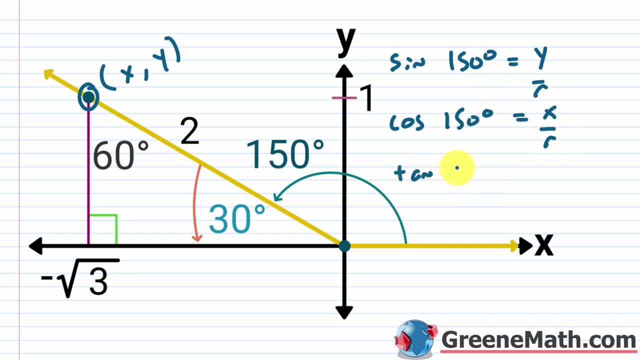 is x over r, And then we have tangent of 150 degrees. This is y over x. So we'll look at this in a moment and we'll compare it. Now. I want you to notice that you have this reference angle here, which is 30 degrees right. Again, if you're in quadrant two, you have this entire guy here. 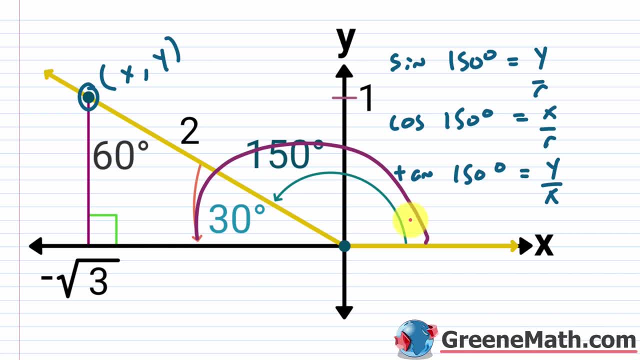 which is a straight angle. that's 180 degrees, And you subtract away the part that you don't want to measure, So that's 150 degrees. So 180 degrees minus 150 degrees is your 30 degrees, So that's the amount of the rotation left to get from the 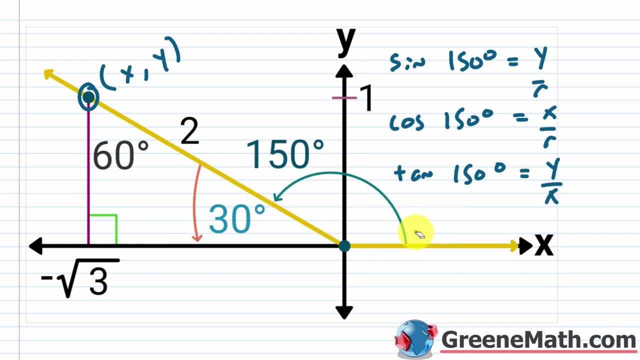 Terminal side to your x-axis. Okay, So I want you to think about: what would the x value be? What would the y value be? What would the r value be? So the r value is simple, It's just going to be two. So r is equal to two. For your y value, again opposite of the 30 degree angle, this side, 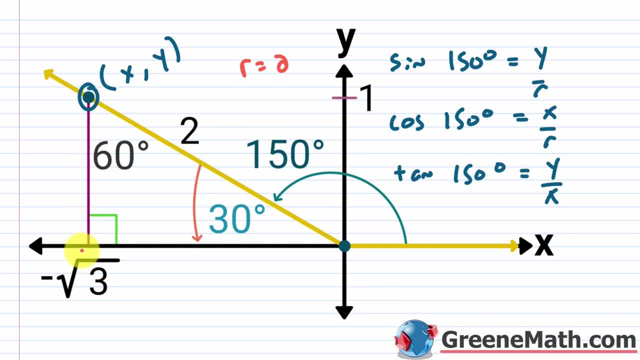 has length one. So if I'm starting here and going here, well, I've traveled one unit up And again you see the one right there. So the y value here is going to be one. When we think about the x value, notice that we're. 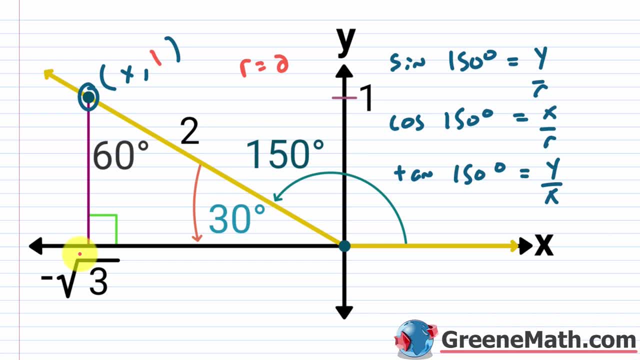 Going left right. If we go to the left of the origin on the coordinate plane the x values are negative. So this length right here, we know that side adjacent to 30 degrees is length square root of three. But again because we're on the coordinate plane, 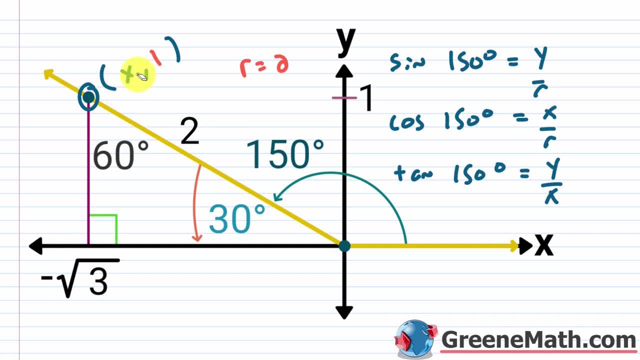 this is the negative of the square root of three for this x coordinate right there. So let's put this right here. So the negative of the square root of three, like that. Okay, So let me actually write this all out. So the x value here is the negative of the square. 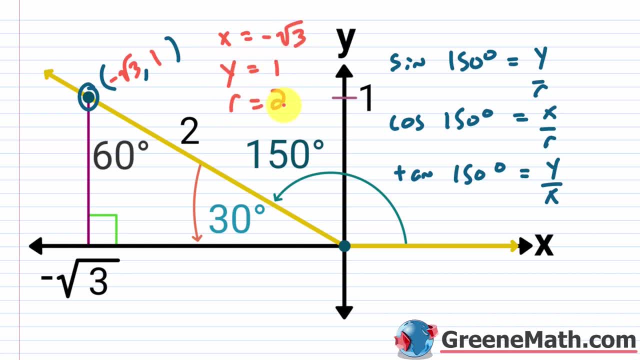 root of three. The y value here is one And the r value here is two. We're going to think about these values here and then we're going to compare them to these trig function values for this reference angle, which again is 30 degrees. So we have y over r, So y is one. 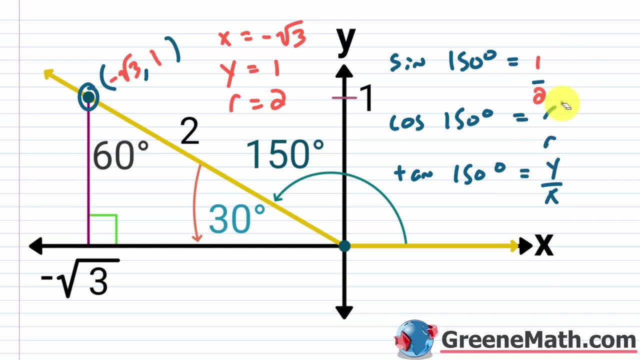 and r is two. Then here we have x over r, So x is the negative of the square root of three over r, which is two. And then here we have y over x, So y is one and x is the negative of. 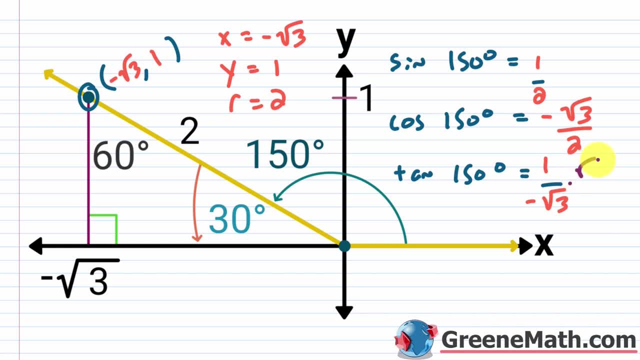 the square root of three. So let me actually rationalize the denominator here. So times the square root of three over the square root of three. So this would be the negative of the square root of 3 over 3.. Now I want you to think about these function values that we talked. 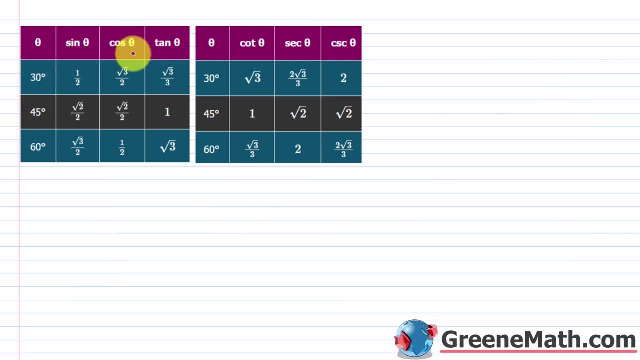 about With a 30 degree angle, the sine of theta is a half, the cosine of theta is square root of 3 over 2, and the tangent of theta is square root of 3 over 3.. So, coming back here, you'll see that. 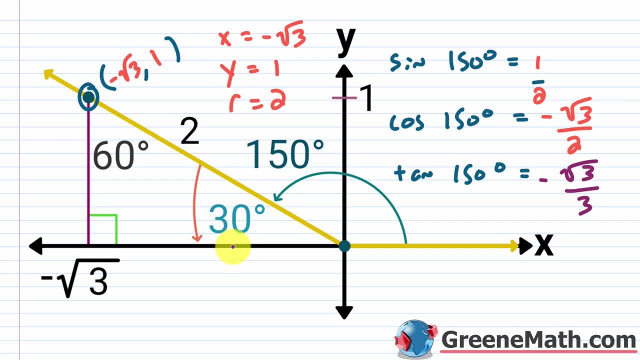 everything matches in terms of absolute value. Okay, so this leads to an important result. What's going to happen is, if you want to find something in quadrants 2,, 3, or 4, you just first find the reference angle. Okay, so, if it's a reference angle of 30 degrees, 45 degrees or 60, 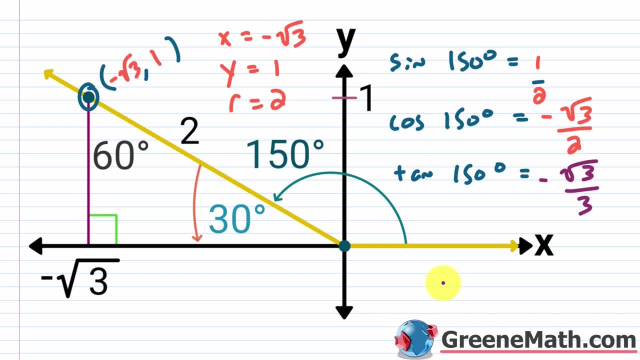 degrees. you can use a little table. We'll talk about other values later on, but for right now that's what we're going to work with. So that's your first step. So you would figure out, in this case, what is the sine of 30 degrees. Then you would apply the appropriate sine based on your 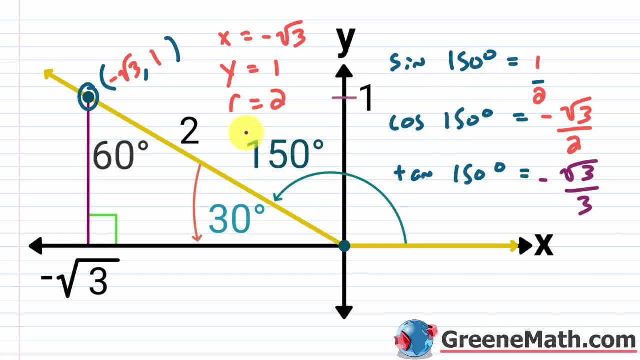 sine rules right. So we know, in quadrants 1 and 2, sine is positive. So here the sine of 150 degrees is a half, because again the sine of 30 degrees is a half And it's going to be positive in quadrant 2, so you don't have to make a sine change there. 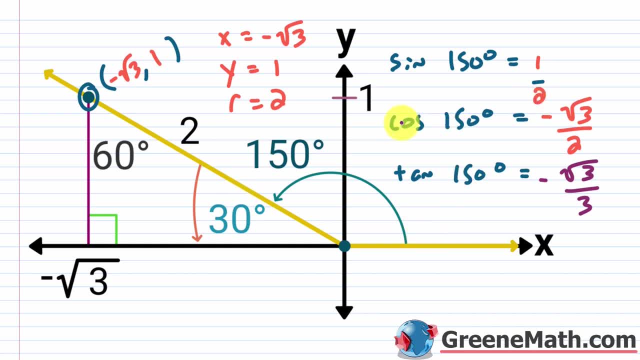 But in quadrant 2, cosine is negative, right? So that's why the cosine of 30 degrees, which was the square root of 3 over 2, is not going to exactly match the cosine of 150 degrees. You have to apply that negative there to account for the fact that cosine is negative in quadrant. 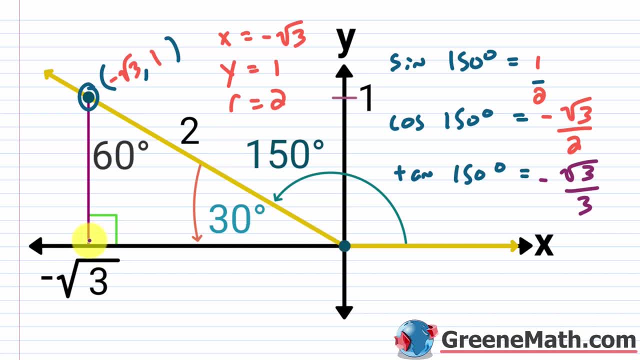 2, because in this case your x values are to the left of the origin and so they're going to be negative. Then we think about the tangent of 150 degrees, Again in quadrant 2, you're going to be negative for your tangent value, So you have to take your tangent of 30 degrees, which is 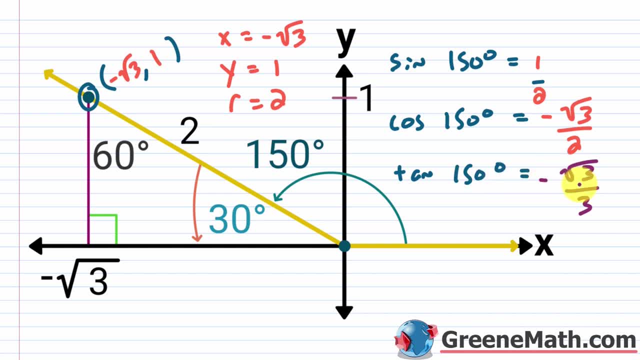 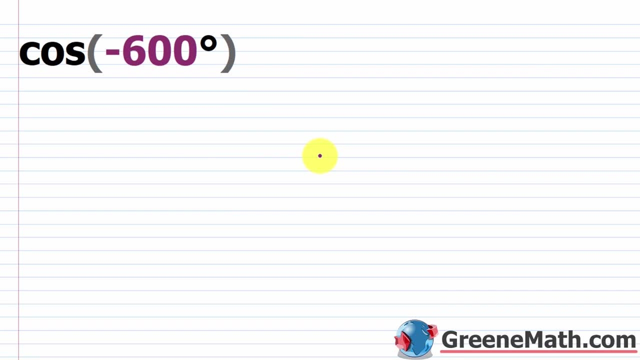 square root of 3 over 3, and then slap the negative on there to get your answer here. So let's go ahead and take a look at some examples. All right, so we're going to start out with cosine of negative 600 degrees. So again, I'm going to first find the coterminal angle. 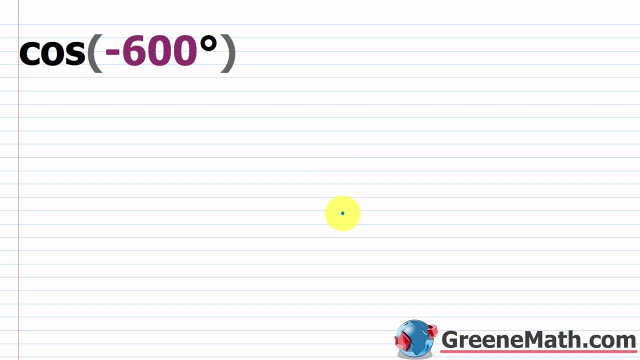 between 0 degrees and 360 degrees, just to make my life easier. So let me put negative 600 degrees. I'm going to need to add 720 degrees to that, So that's going to give me 120 degrees. So this is. 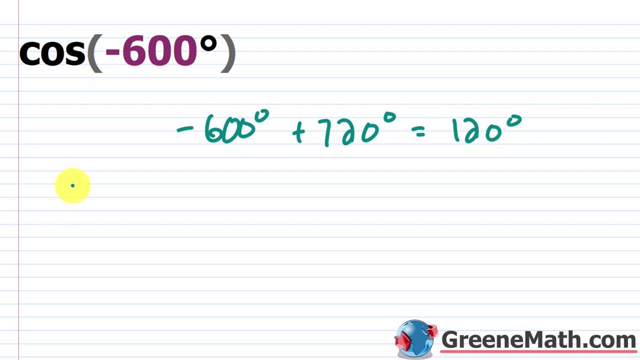 what I'm going to work with. So the first thing is, if I have a 120 degree angle, my theta prime, which is my reference angle, is going to be again. I'm in quadrant 2, so 180 degrees minus. 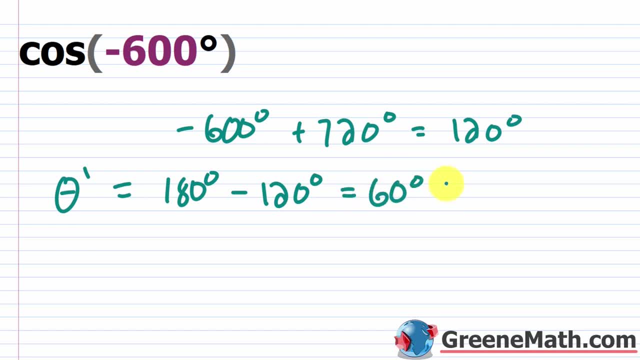 120 degrees, which is 60 degrees. So this is my reference angle. Let me write: theta prime is equal to 60 degrees and we can erase this scratch work. Cosine of negative 600 degrees is equal to the cosine of this 120 degrees. Now here's where you have to find the coterminal angle, which is 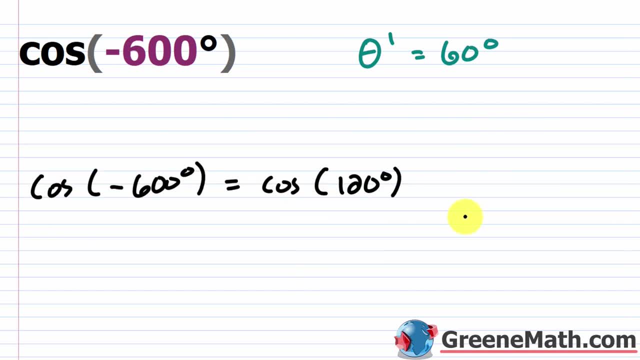 negative 600 degrees. So what I'm going to do is I'm going to go ahead and I'm going to apply a little bit of thinking And you want to say: well, this is in quadrant 2, is cosine positive or negative? It's negative in quadrants 2 and 3.. So I'm going to put equals here and then I'm going 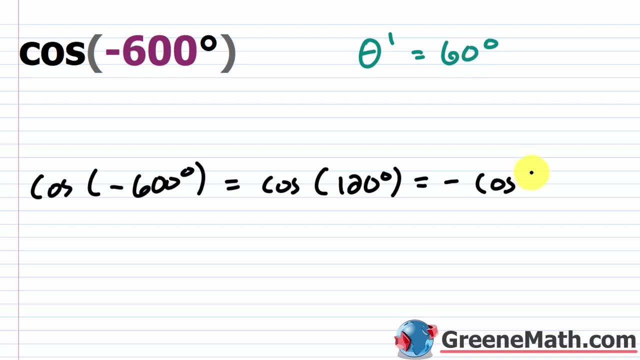 to put the negative of the cosine of this reference angle, which is 60 degrees. Remember, when you talk about things in quadrant 1, so the 30 degrees, the 45 degrees or the 60 degrees, everything is positive, right? All students take calculus In quadrant 1, they're all positive. So that's why. 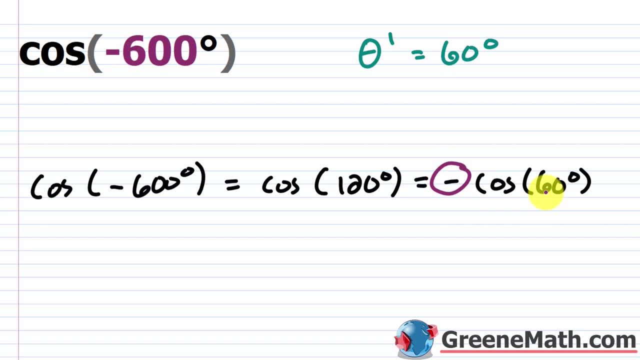 it's negative here to this result. So the cosine of 60 degrees, if you go back to your table, is going to be 1 half. So what we'll do is say this is equal to the negative of, again, the cosine of. 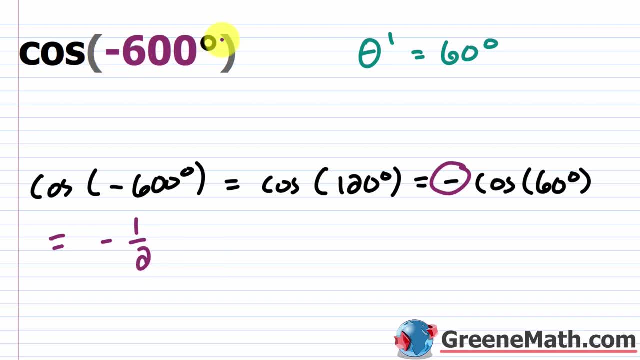 60 degrees is a half. So your answer here for the cosine of negative 600 degrees is going to be negative 1 half. Okay, let's look at one more. So here we have the secant of 495 degrees. So again, 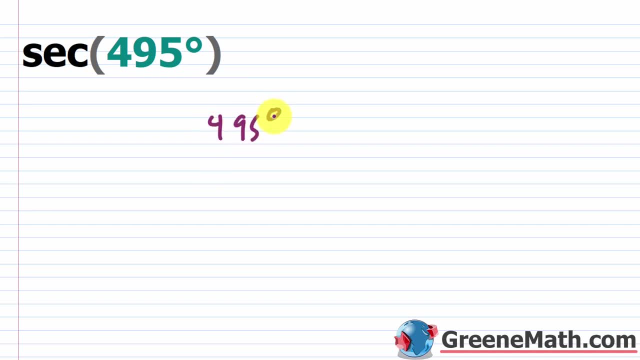 I would first find my coterminal angle. So 495 degrees. Let's subtract away 360 degrees And that's going to give me 135 degrees. So when I think about 135 degree angle again, I'm going to be in quadrant 2.. And my reference angle, my theta prime, is 180 degrees. 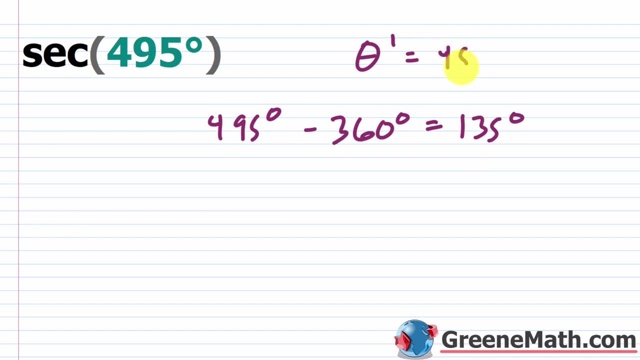 minus 135 degrees, which is 45 degrees. Okay, so that's what I'm working with there. So let me get rid of this And I'll just state that the secant of this 495 degree angle is equal to the secant of this coterminal angle, which is 135 degrees. So this is equal to. 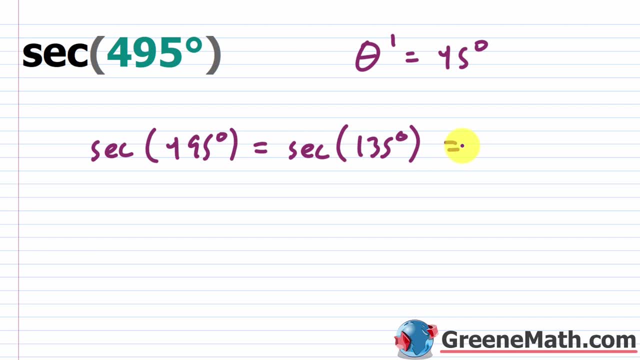 if I'm in quadrant 2, secant is going to be negative, right? Remember, secant is the reciprocal of cosine. They're both going to be negative in quadrants 2 and 3.. So I'm going to put this negative out in front to account for that, And then I'm just going to think about. 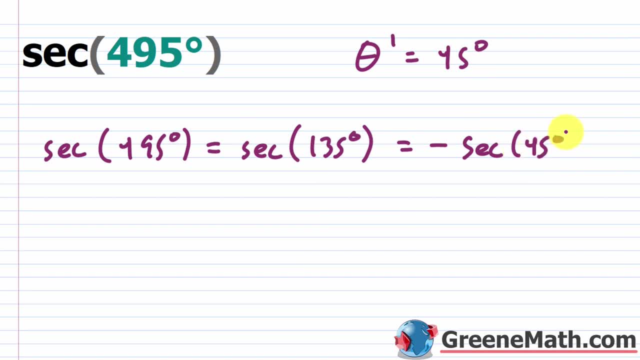 the secant of 45 degrees. So, coming up to my table, if I want the secant of 45 degrees, it's going to be the square root of 2.. So I'll say this is equal to: don't forget your negative. 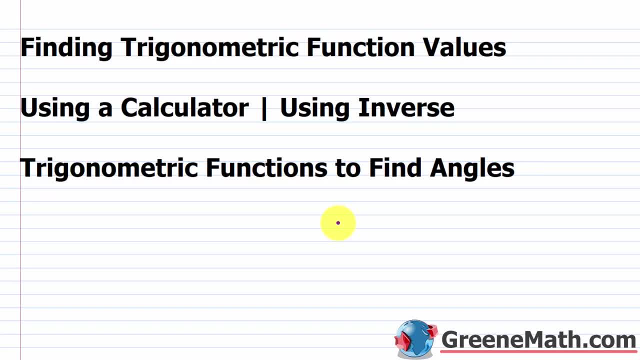 so the negative of the square root of 2.. In this lesson I want to talk about finding trigonometric function values using a calculator. We'll also discuss using inverse trigonometric functions to find angles. Okay, so the first topic here is: 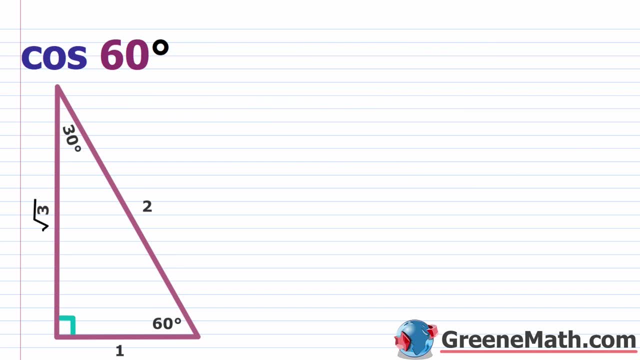 going to be very, very simple. I just want to make sure everybody's on the same page with using their calculator. If you're using an online calculator, you could pretty much just skip this part of the lesson. If you see something like the cosine of 60 degrees we already know from this special 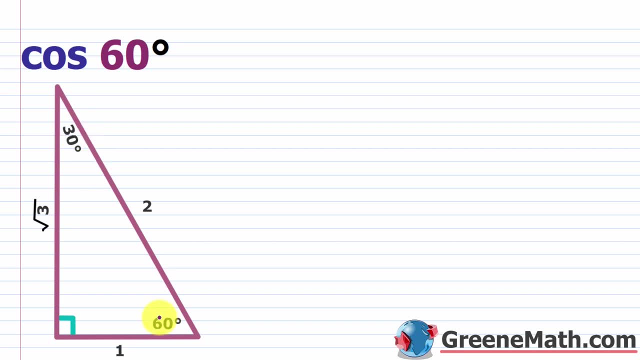 right triangle, where we have 30 degrees, 60 degrees and 90 degrees. If we want the cosine of 60 degrees, well, it's adjacent, which is one over the hypotenuse, which is two right As a. 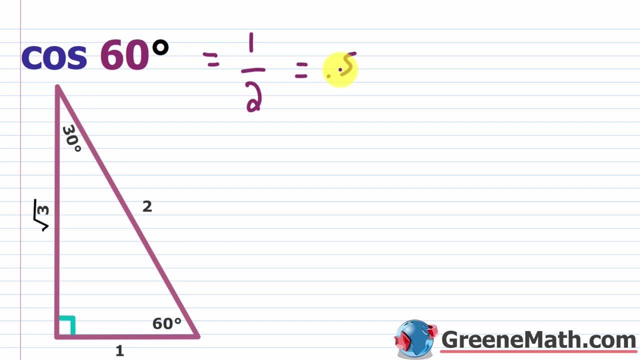 decimal, this is 0.5.. So what I want everybody to do is pull out their calculator that they're going to use for this course, And it should have a sine key, a cosine key and a tangent key. you want to figure out what mode you're in first. So most calculators have a radian mode. we're going to 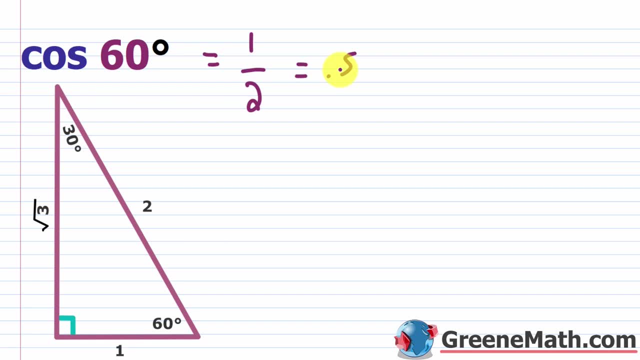 talk about radians later on- and a degree mode. you want to select degree mode, So you should be able to use the cosine key on your calculator, So it would look like that, And then basically, you would have some parentheses that would open up and you just want to type in 60. Don't worry about trying to find the degree. 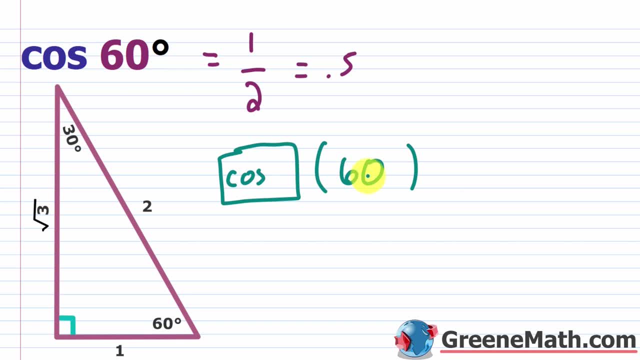 symbol. If you're in degree mode, then it knows you're working with 60 degrees, So you hit the enter key after that. So you hit your enter, your enter key after that, and you should get a result of 0.5.. If you're not, 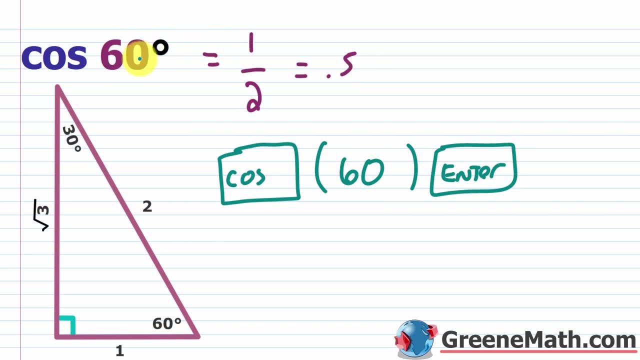 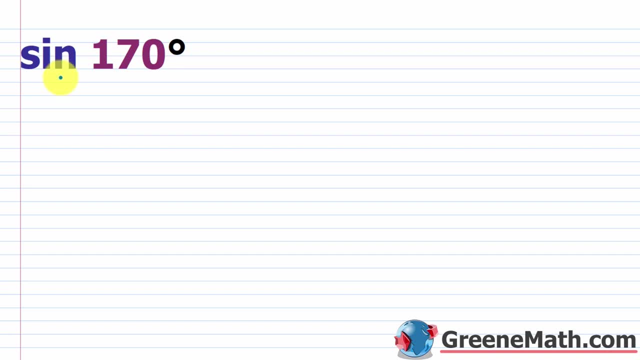 again, just making sure you're on the same page with me. So we have the sine of 170 degrees, So I would just hit my sine key. I would just hit my sine key and then in the parentheses type in 170.. And then you're going to hit your enter key And this should give you, let's say, approximately 0.1736481777.. That's where my calculator cuts off. Usually the book will tell you. 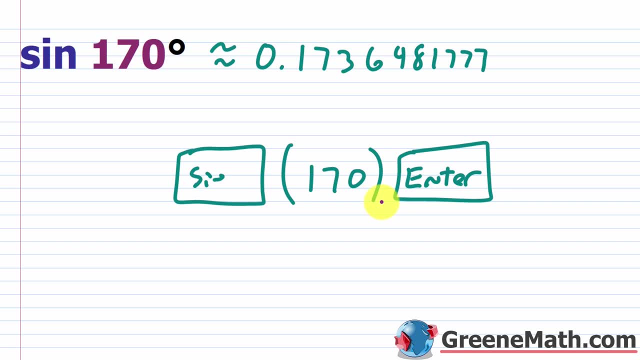 where they want you to round to. So let's just say we want to round to the nearest 10,000.. So that's four decimal places, So 1234.. Remember, this is the tenths, the hundredths, the thousandths. 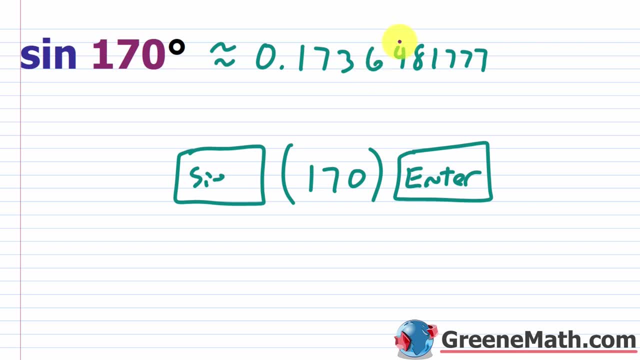 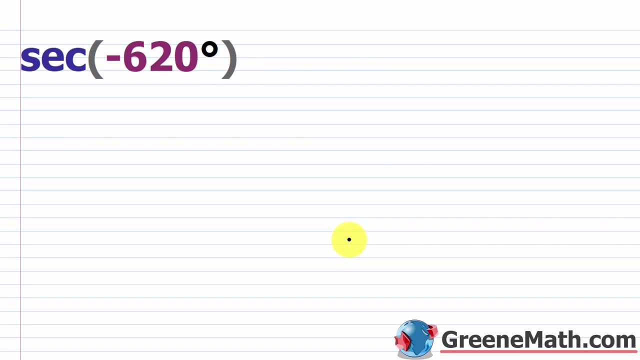 and this is the 10,000.. So, if I think about it, the digit that follows is a four, so the six would be unchanged And you could just get rid of all these digits that follow. So the sine of 170 degrees is going to be approximately 0.1736.. All right, let's take a look at another example. 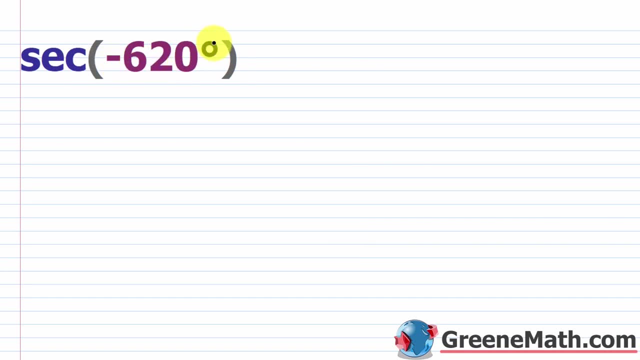 So here we have the secant of negative 620 degrees. Now there's a few things here. First off, you might not have a secant key on your calculator. The calculator I use does not have a secant key, So you would say the secant of some angle theta again using your reciprocal identity. 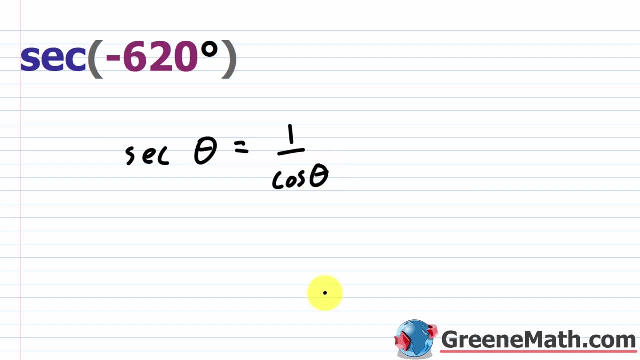 you could say: this is one over the cosine of theta, since most calculators do have a cosine key, So you can convert this over and say this is one over the cosine of this negative 620 degrees. Now another thing you might be concerned with. you've seen throughout the course. 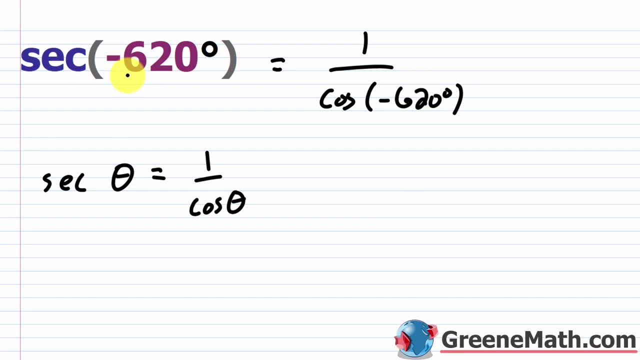 if I got a negative angle or an angle whose measure was greater than 360 degrees, I would always find the coterminal angle between zero degrees and 360 degrees. Now you could do that, But if you're using a calculator, you don't have to. 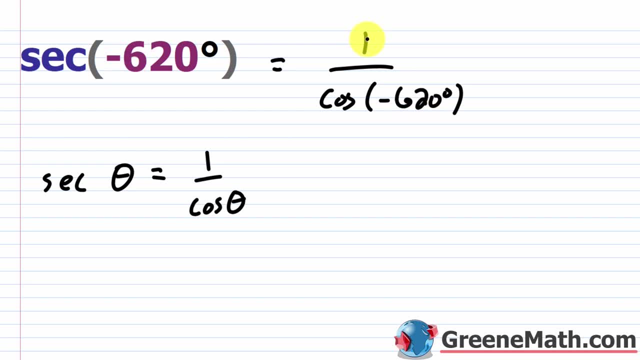 this will automatically calculate the value for you. So you're just going to type one, then the divided by key, hit your cosine key. When the parentheses come up, just type in negative 620.. Again, don't worry about the degree symbol hit. 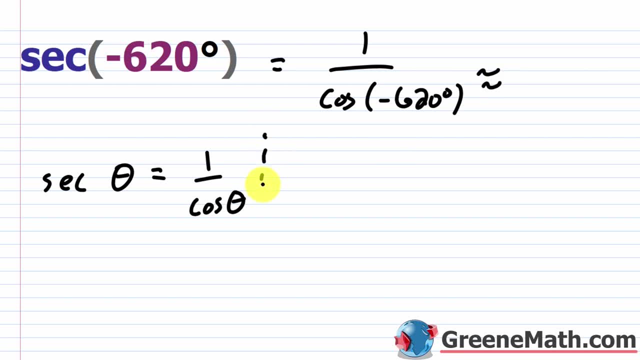 enter And we're going to get approximately. we just make a little border here. If I pick up my calculator, I'll say it's negative 5.75.. And then I'm going to have 8770483.. Now, with this guy, 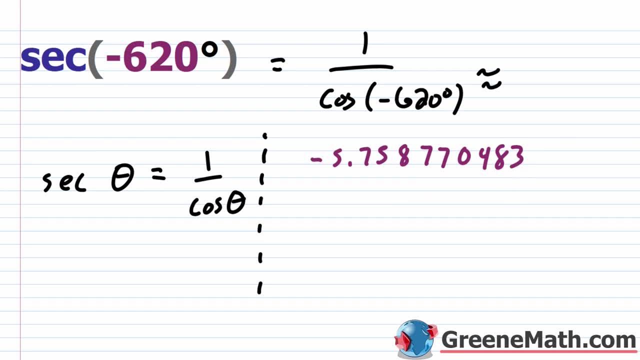 again, if you wanted to round to the nearest 10,000, that's pretty common for most books. Let's see, we have the tenths, the hundredths, the thousandths and then the 10,000. So this: 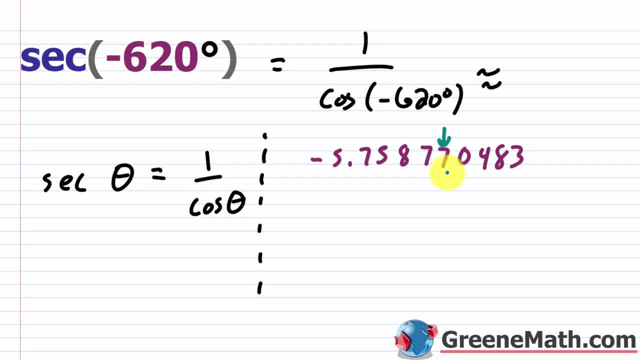 is the digit that follows, So the 7,000, the hundredths, the thousandths and then the 10,000.. falls in the category of five or greater. So I would add one to this seven and then I would cut. 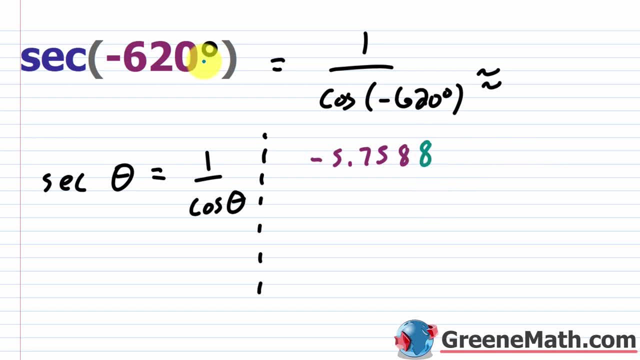 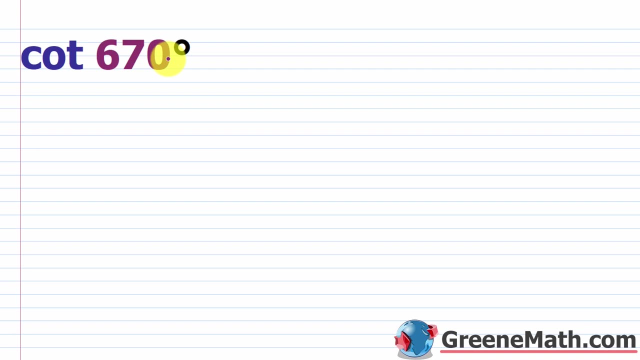 all these off, So this will turn into an eight. So your answer here for the secant of negative 620 degrees is going to be approximately negative 5.7588.. Okay, let's look at cotangent of 670 degrees. So again, you might not have a cotangent key, but more than likely you have a tangent key. 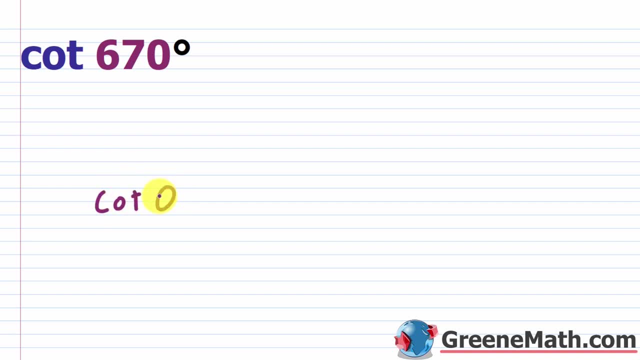 So again from the reciprocal identities, the cotangent of theta is equal to one over the tangent of theta. So really you could just say this is equal to one over the tangent of your 670 degrees, like this, And again you could just follow those steps with your calculator. 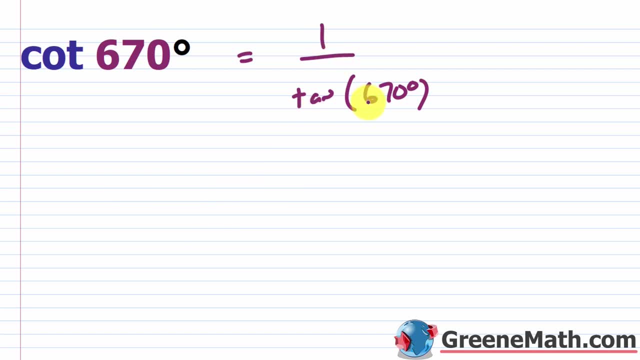 hit one hit divided by hit your tangent key inside the parentheses, type in 670, and then close the parentheses and hit enter. And so this is going to be approximately, let's say, negative. I'm going to go 0.839099.. And then we'll have 6309.. 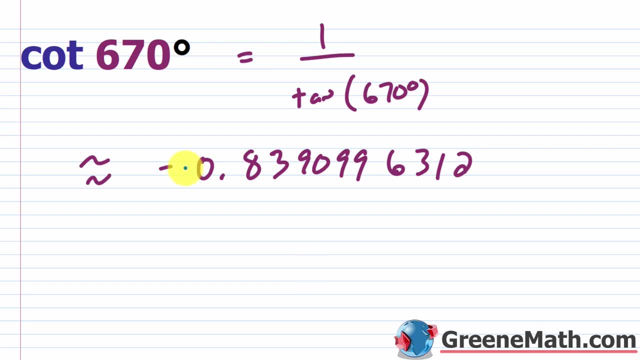 And again, if you wanted to round to the nearest 10,000, again, forget about the fact that it's negative. I know that throws off a lot of people. you've got 1234 decimal places, So this guy right here- the digit that follows is a nine, So add one to the zero. that's going to be one. And then 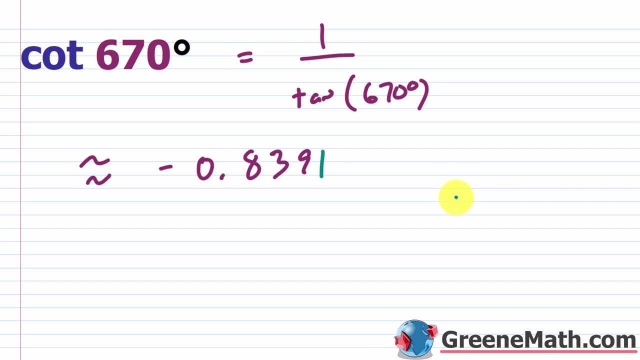 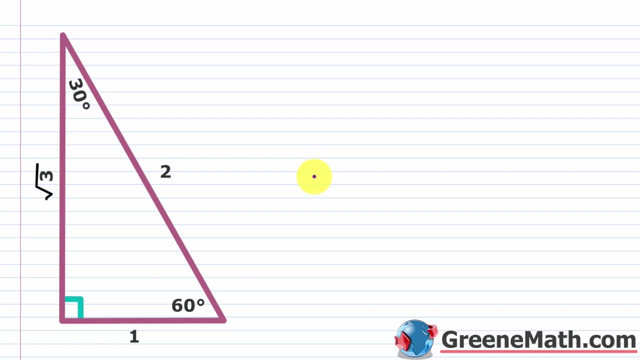 you can cut all these digits off. So, rounding this to the nearest 10,000, you're going to have negative 0.8391.. All right, let's spend a little bit of time now introducing the inverse trigonometric functions. So these are going to be a little bit confusing, but they're going to be a little bit. 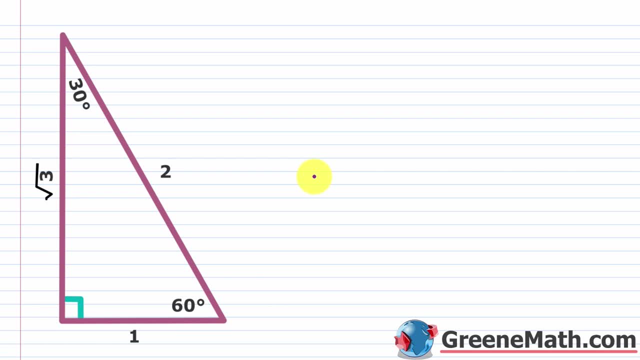 confusing. So these are going to be a little bit confusing, but they're going to be a little bit confusing For right now. when we get further into the course, we're going to spend a lot of time developing the whole thought process behind how and why these guys are going to work For right. 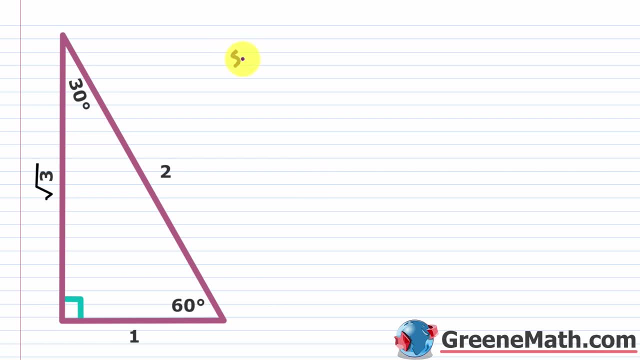 now. I just wanted to think about something simple. Let's say, you had the sign of 30 degrees And again we have our special right triangle here, So we can immediately see that the opposite is one and the hypotenuse is two. So we know this is one half. And again you can type that: 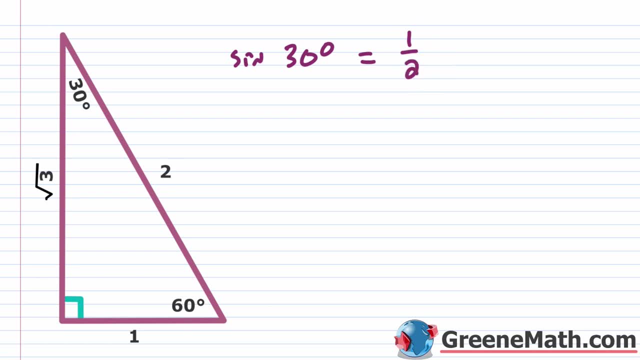 into your calculator and verify, you would get point five or half as a decimal. Now what if you typed into your calculator sine inverse? so it's going to look like that, where you might see arc sine. that's another way to denote it. But basically, if you took this part, 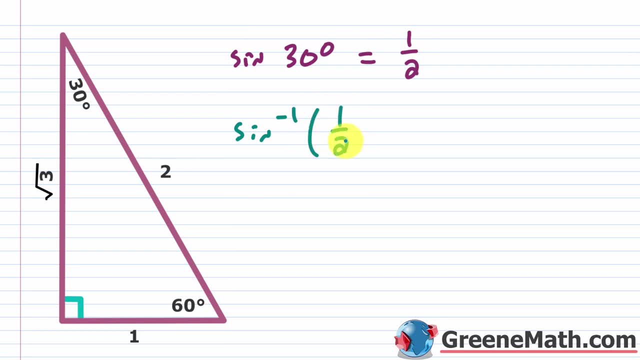 right here, or your answer from this. so let's say- I put that in the parentheses- this is going to give you this angle measure back. So in other words, it's undoing what you did here. Here you took sine of your angle, which is 30 degrees, and you want to find the opposite over the 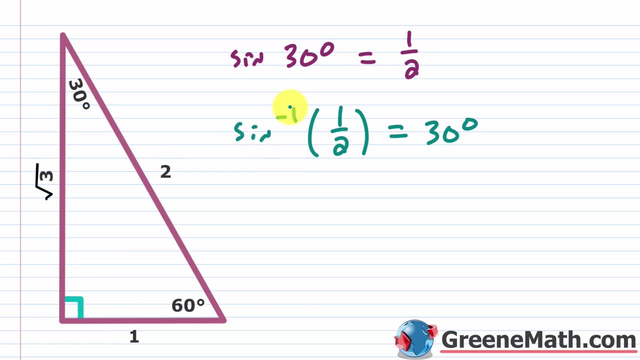 hypotenuse. So that gave me a half. Here you have the inverse trigonometric function and you want to take your sine and you're taking your opposite over your hypotenuse and it's going to kick your angle measure, which is 30 degrees back out to you. So in other words, you could say that you 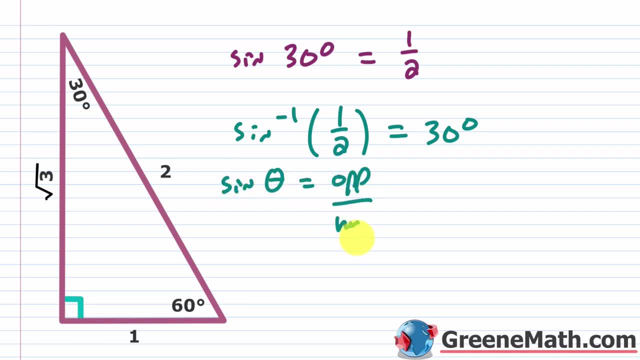 have sine of theta is the opposite- over the hypotenuse And in this case you have the sine inverse, which is going to be you plugging in the opposite over the hypotenuse and you're going to get your angle theta back. But there's a problem here, Okay, and it's kind of a big problem. But 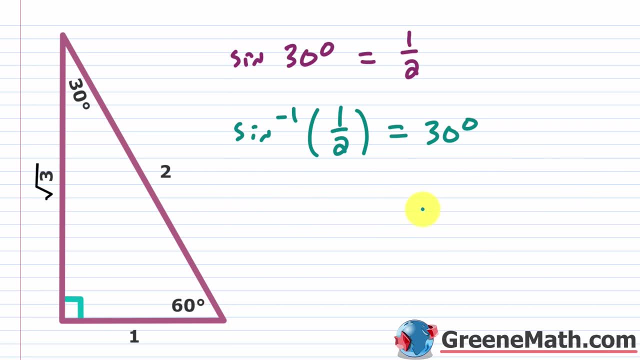 again. we'll talk about this more later on in the course. If you typed into your calculator sine in, let's say, sine of 390 degrees, So this is an angle that's coterminal. with 30 degrees, it's going. 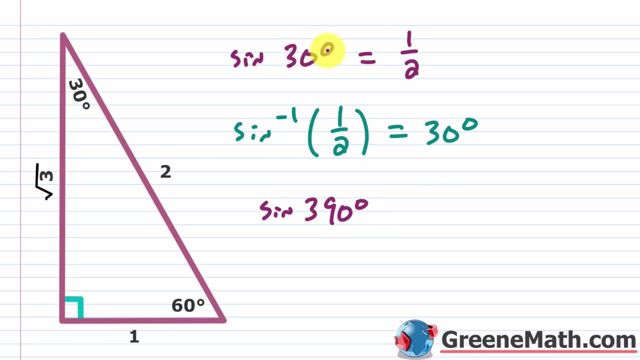 to be in the first quadrant and it's going to have a reference angle of 30 degrees. Well, you would get point five or one half. Now I just saw that if I did sine inverse of one half, I get 30. 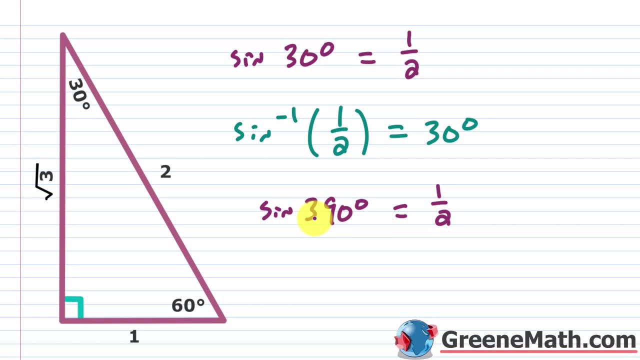 degrees. So I'm not getting my 390 degrees back that I'm looking for. So what's going on? Well, the problem is that sine is not a one to one function. We talked about this earlier in our pre calculus course, where, for a one to one function to exist, you have to. 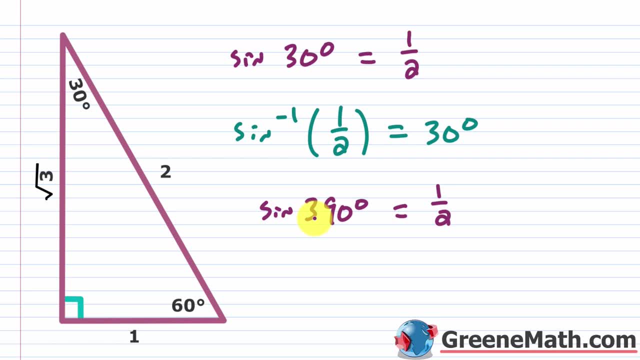 have, for each x value a given y value and for each y value a given x value. So for each x there's one y And for each y there's one x. Well, that's not going to be true with your sine. 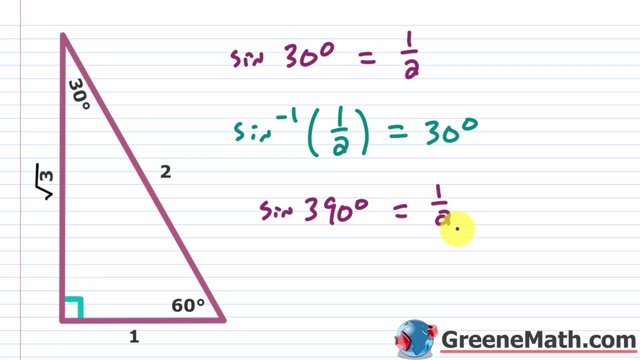 function. So what happens is you have to restrict the domain in order to make it a one to one function, And that leads to the fact that if I plugged in one half here, I'm only going to be able to get something in quadratus. So I'm going to have to restrict the domain in order to make it. 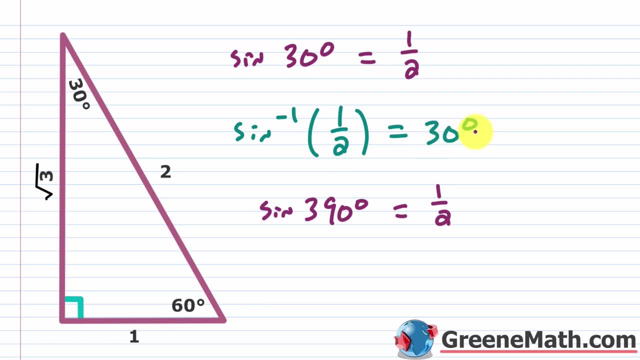 one, So that's 30 degrees. If I needed to find something else, well then I'm going to use the concept of a reference angle And I'm going to think about where sine is positive. So, in other words, I know that sine is going to be positive in quadrants one and two, So really anywhere in 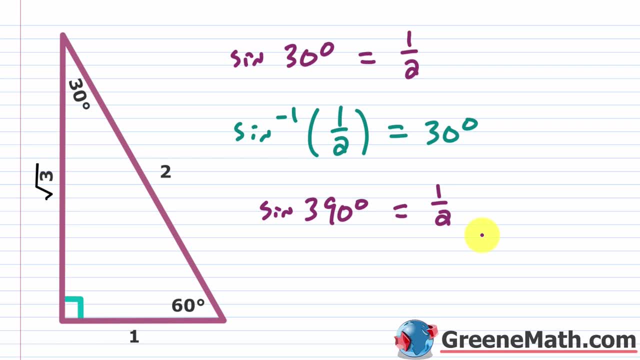 quadrants one or two where I would have a 30 degree reference angle. well, basically, my sine value is going to be a half. If I did sine of, let's say, 150 degrees, that has a 30 degree reference angle. So that's going to be a half. 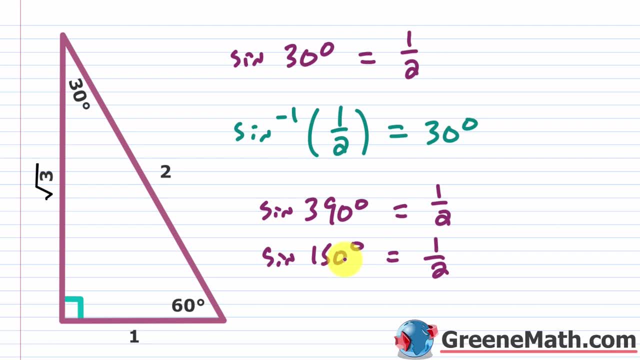 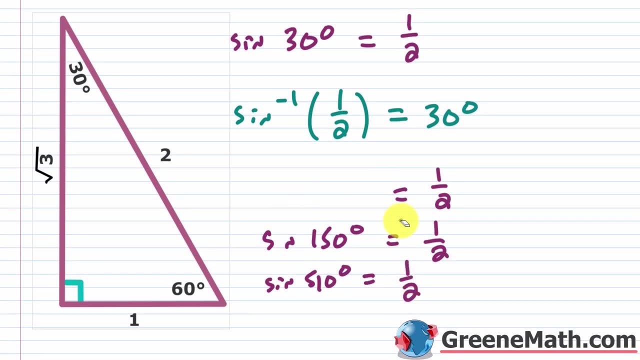 If I added 360 degrees to that, I would have 510 degrees, And if I did the sine of 510 degrees I would also get a half, so on and so forth. So if you ever get a question and we'll see them, 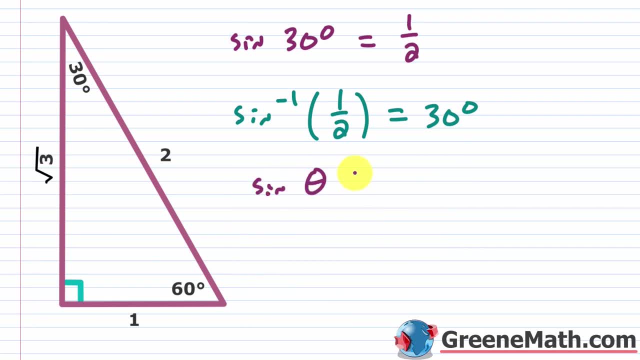 later on in the course where it says something like the sine of theta is equal to a half. well, there's an infinite number of angle measures there where, if you take the sine value of it, you're going to get a half. So, generally speaking, when you see these questions, 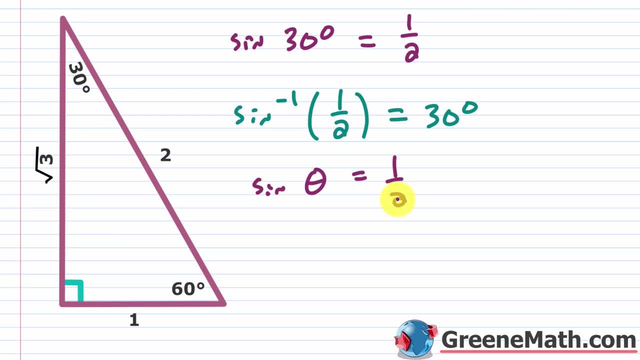 especially in the first part of trigonometry. they're going to tell you that theta is going to be between zero degrees and 90 degrees. So you're going to be in that first quadrant where zero degrees and 90 degrees will be included. So let's look at a little example here. So we have sine of. 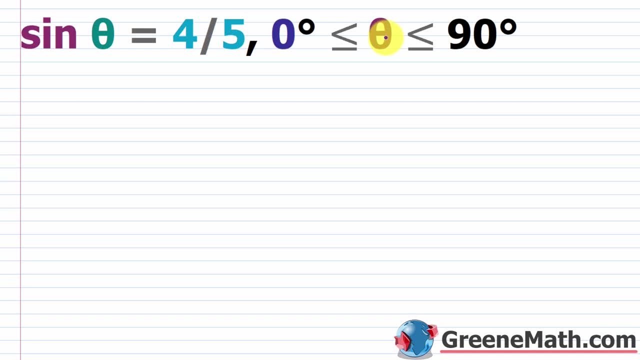 theta is equal to four fifths. And here theta is restricted, like I was just talking about, to be greater than or equal to zero degrees and less than or equal to 90 degrees. Okay, so for this one again we would just use our inverse sine function, So sine inverse of this guy right here. 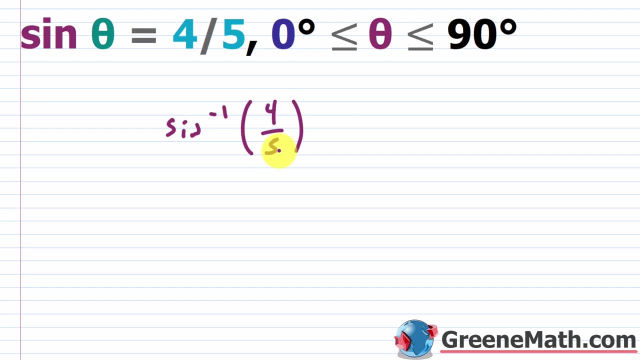 so this four fifths. So it's like I'm plugging in the opposite over the hypotenuse And I'm looking for my theta, And this is going to come from quadrant one. So I'm going to be good to go in terms of this restriction here. So let's punch. 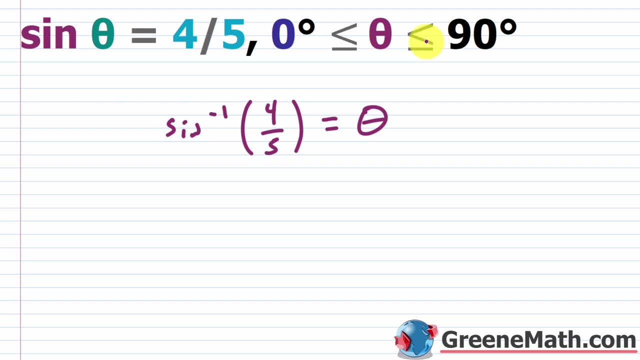 this into the calculator. So hit your inverse sine key, hit four and then divided by five, close your parentheses And let me move this over And I'll say theta is equal to this And I'll say this is approximately. let's write out what we have: So 53.1301, and then 0,2,3,5.. So let's. 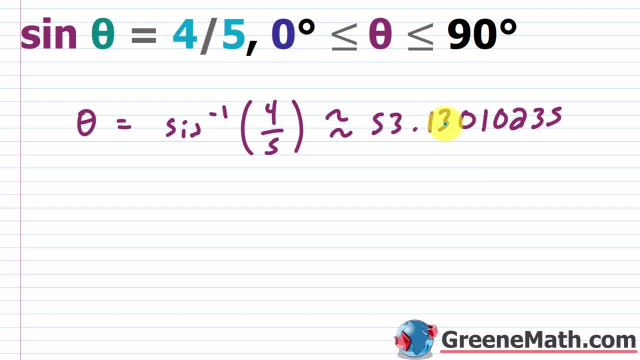 say that's the nearest 10,000th. So you have 10ths, hundredths, thousandths. this is the 10,000th, So the digit that follows is a zero. So we can just cut all these off And this is in. 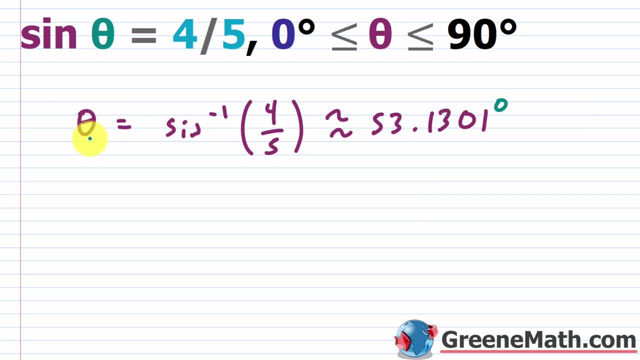 terms of degrees. So our theta here is going to be about, or you can say approximately, 53.1301 degrees. And again, if you didn't have this restriction here, you could really say that theta could be any angle in either quadrant one or quadrant two, where sine is positive, where the 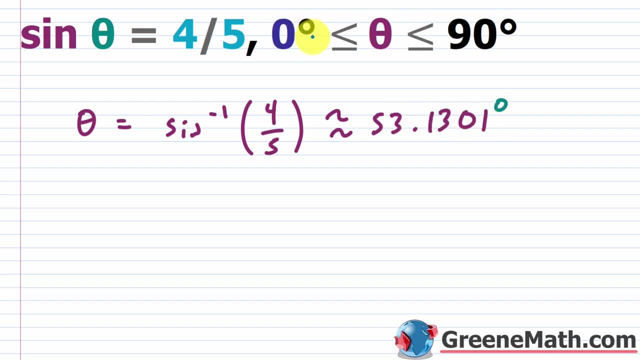 right here, right. so there's an infinite number of solutions. if you take this guy away, this restriction, Alright. so, similarly, we have the cosine of theta. this is equal to two sevenths. So here again, we're going to say that theta is greater than or equal to zero degrees. 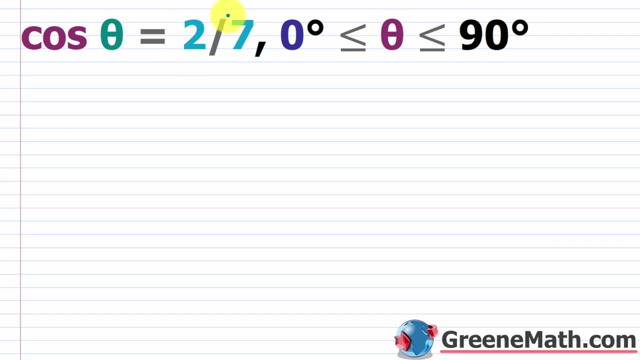 and less than or equal to 90 degrees. So, since this is positive, if we use our inverse cosine function, we're going to get something in quadrant one, so we'll be okay. So I'm going to say that I want my theta to be equal to the inverse cosine, And some people write that as arc cosine, like. 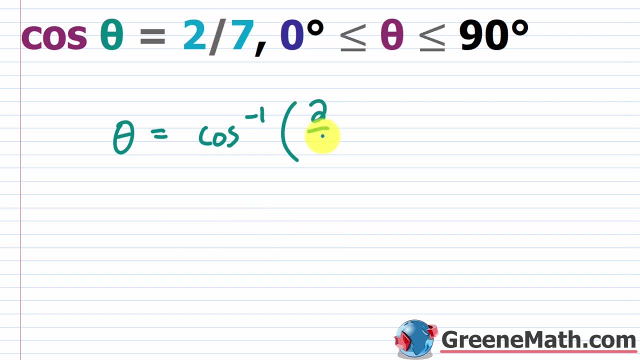 this And basically you're just going to plug this in here. So this two, sevenths, and this is going to spit out my angle, my theta- that will be in quadrant one. So let's hit our cosine inverse button And then, inside the parentheses, type two divided by seven, close your parentheses and hit. 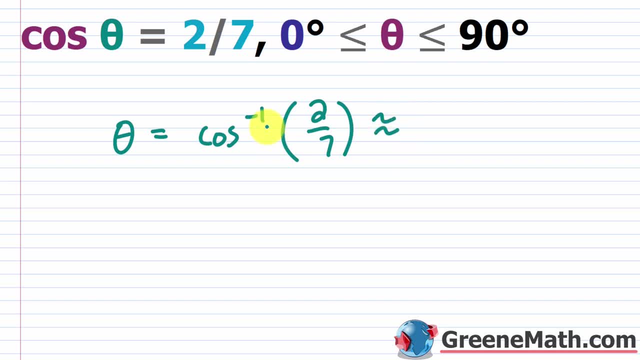 enter. And this is approximately. let's go ahead and say I'll just write out everything: it gives me So 73.3984504.. That's when my calculator stops. If we want to go to the nearest 10,000th, we have the tenths, the hundredths, the thousandths, the ten thousandths. Well, 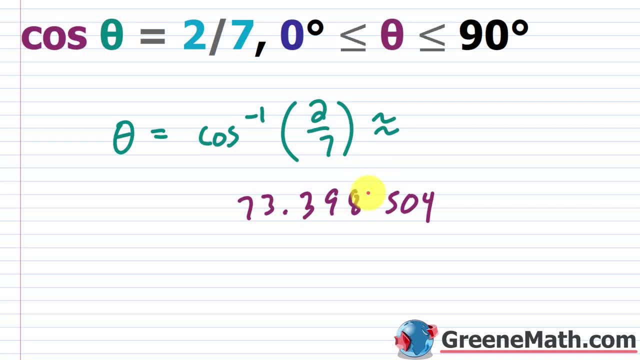 this guy's a five here, So let me add one to this And we'll make this into a five, And then you can cut these off. And this is in terms of degrees. So we would say that our theta here is approximately 73.3985 degrees. Now again, if you did not have this restriction here, then theta could be any. 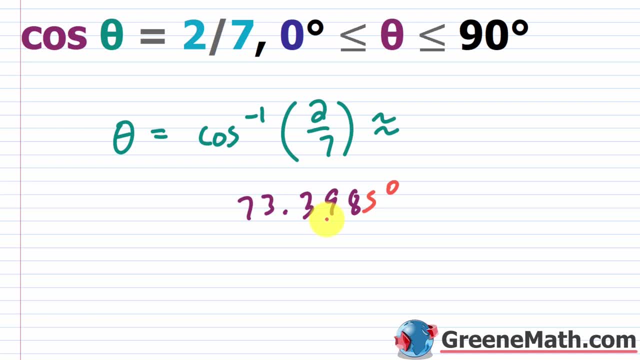 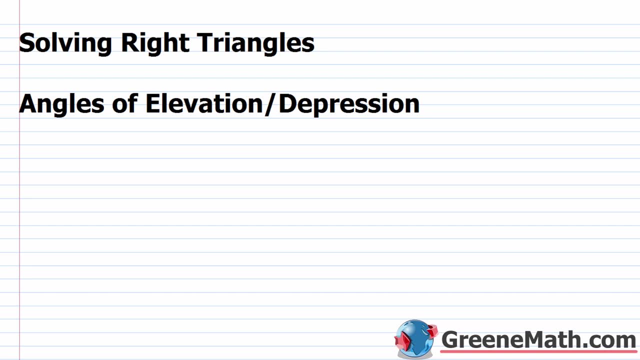 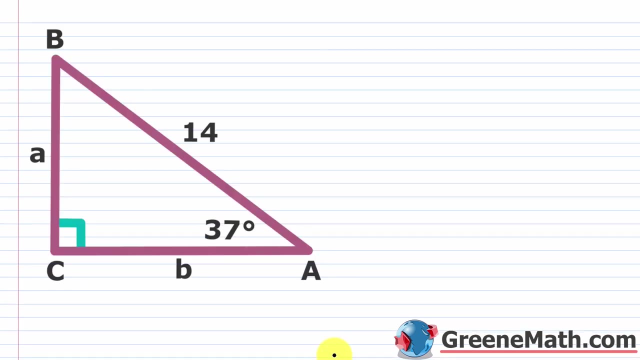 angle that's in either quadrant one or quadrant four. that's where cosine is positive. that has this reference angle. In this lesson we want to talk about solving right triangles and also look at some word problems that involve angles of elevation and also angles of depression. All right, so let's just jump in and look at our first example. 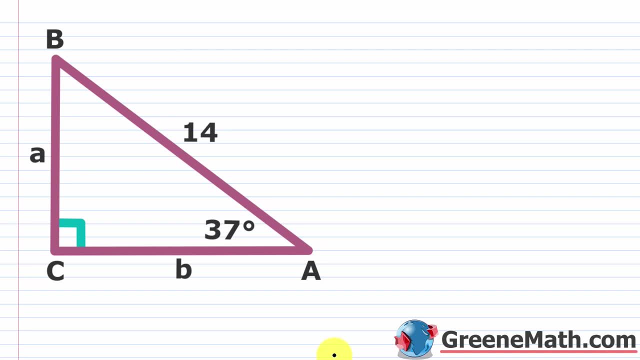 When we talk about solving a right triangle, we're just trying to find all the missing angles and all the missing sides. So in this particular case, we have our triangle here. We're given one side that has a value of 14. And we're going to look at the right triangle And we're going to 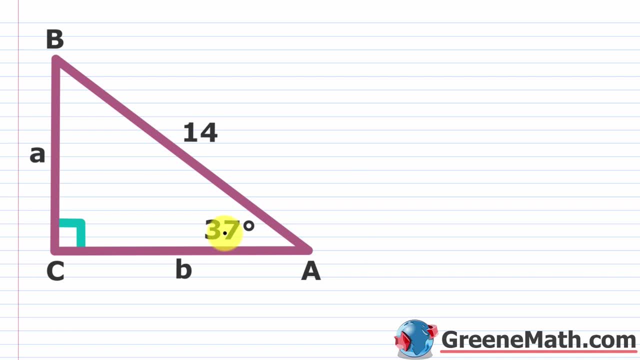 and then we're given one angle with a value of 37 degrees. So I know the measure of angle A is 37 degrees. I know the measure of angle C- because it's a right angle- is 90 degrees. You can write: 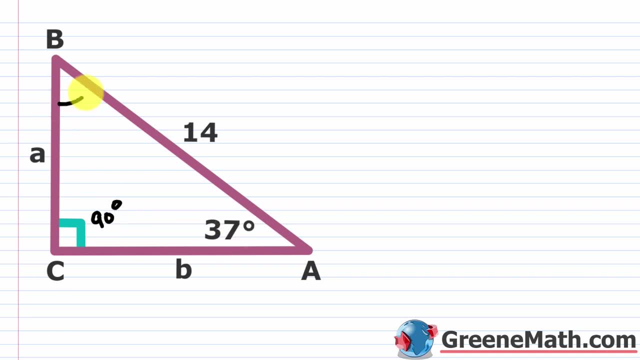 that in there, And so if you wanted to figure out what the measure of this angle is, well, you know that the sum of the three angles is 180 degrees. So you could say that 180 degrees minus your 37 degrees, plus 90 degrees- this guy right here- would be the measure of your angle. 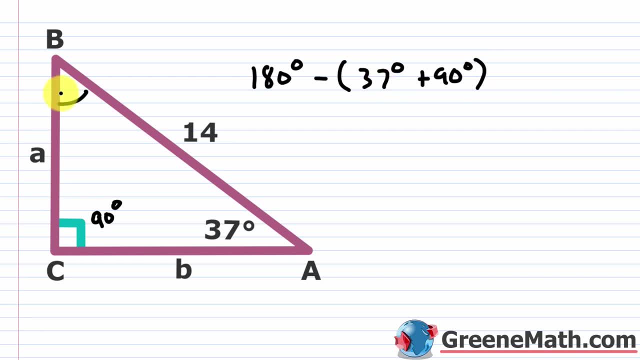 B. So let's go ahead and crank that out real quick. So 37 degrees plus 90 degrees is 127 degrees, And if I subtract 180 degrees minus 127 degrees I get 53 degrees. So the measure of this angle. 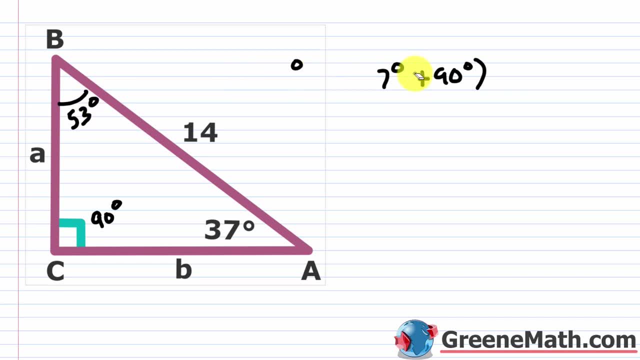 here is going to be 53 degrees. Okay, so you can write it like this, where some people will say that the measure of your angle B is equal to 53 degrees, like this: So, whatever notation your teacher prefers, that's how you want to give it. So I'm just going to erase this. 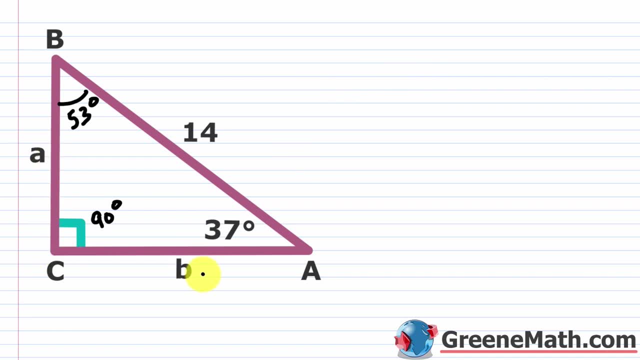 so we have some room, All right. so now we want to find these missing sides. So we have this guy right here and this guy right here, Okay. so I always use the information given so that I can get a more accurate answer. In almost every case, you're going to have to round Okay and just get. 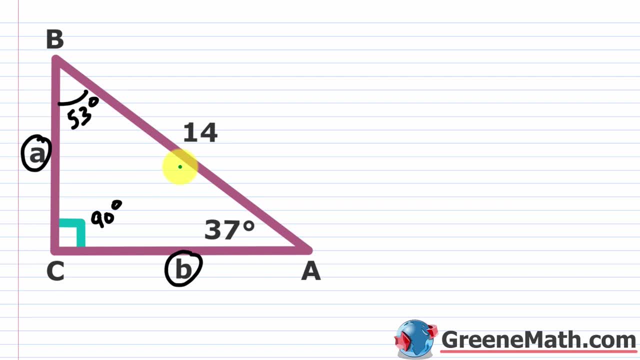 with your teacher or your assignment to know what you need to round to. So for these guys, I'm going to round to the nearest 10th. just to keep it really simple, I'm going to start with the fact that I was given this angle here, which is 37 degrees. Okay, so I know that some of these angles are 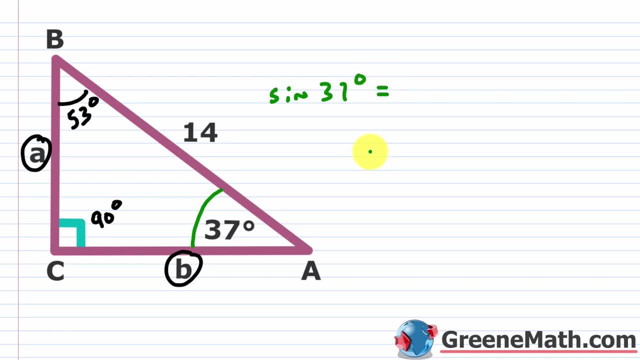 going to be lowercase. So, for this line of 37 degrees is equal to what It's opposite. it's opposite over hypotenuse. Okay, so the opposite side here is this lowercase, This lowercase a, and the hypotenuse here is given as 14.. Remember, the hypotenuse is always across from your right. 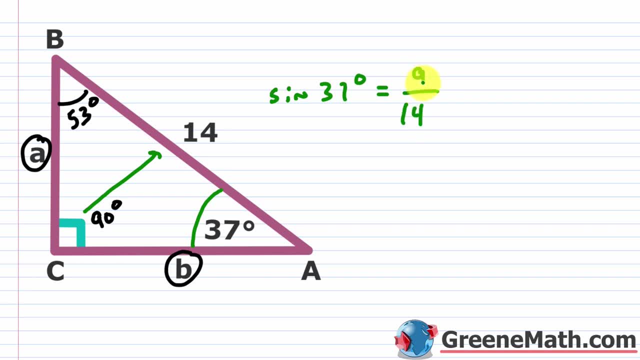 angle. Okay, so this guy is going to be 14.. Okay, so how can we solve for this a here? okay, the lowercase a. we just multiply both sides by 14 to clear the denominator Okay, and then we're going to. be able to get a more accurate answer here. So in this case, we're going to solve for this a: okay, we're going to write this in the upper case, Okay, the hypotenuse at the right corner, and then we're going to write. 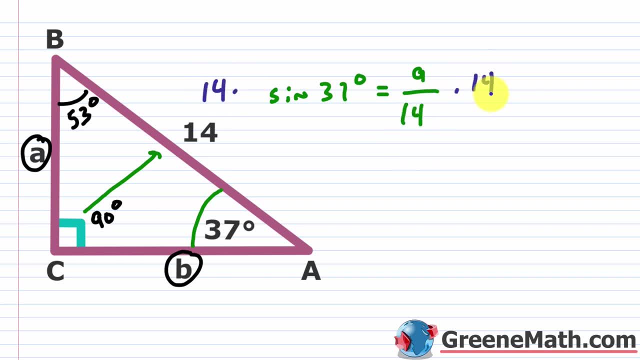 okay, so we'd multiply by 14 over here and by 14 over here, and this guy cancels with this. okay, same thing we'll be doing forever. so what is 14 times sine of 37 degrees? well, if you punch that up on your calculator, you're going to get about 8.4 again if we go to the nearest tenth. so this: 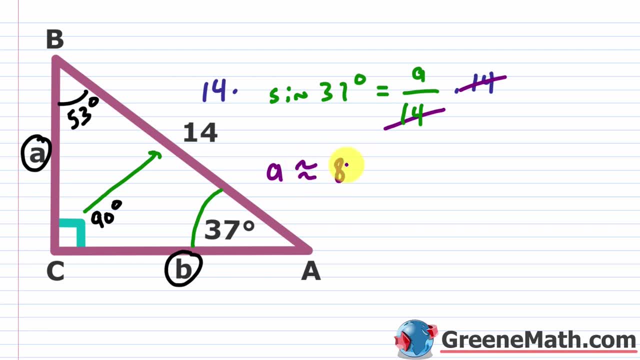 guy right here. i'm just going to say that a is approximately 8.4. okay, so it's approximately 8.4, and i'm just going to write in that it's 8.4 here again, we know this is an approximation, okay, so what about this lowercase b here? what's that going to be again, when you work with these? 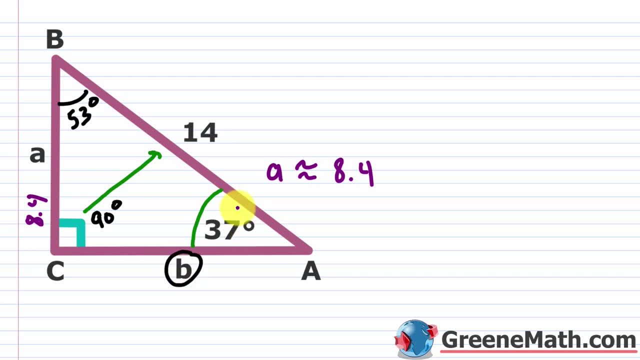 problems. try to use the information that you're given, because in some cases you're going to have to approximate your angle, so you won't have this guy available to you as an exact measure. so i'm going to go with the 37 degrees that they gave me and i want to think about how can i get this guy. 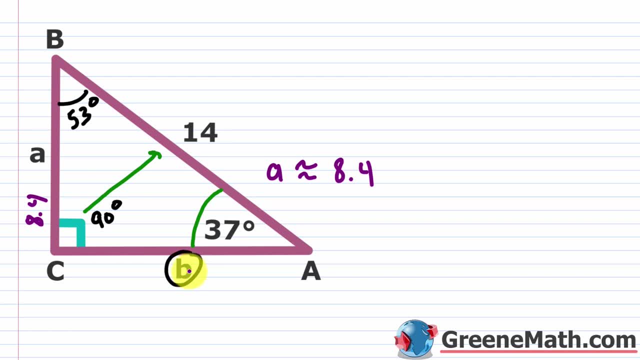 right here. so we would use cosine now because the the cosine of the angle is going to be 8.4 and the cosine of the angle is going to be 8.4. the cosine of the angle is going to be 8.4. so we're going to use cosine now because the 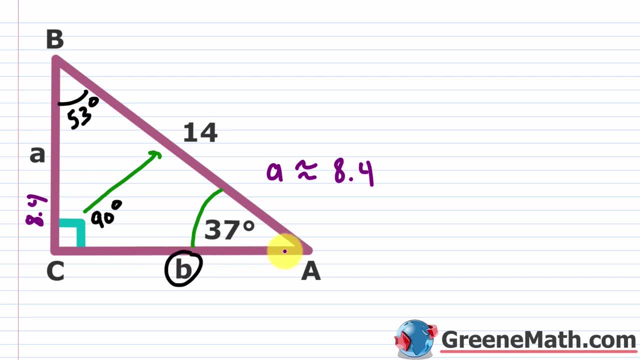 side here, which is lowercase p, this guy is the adjacent side and this guy is the hypotenuse. So if I did cosine, okay, cosine of 37 degrees, well now this is equal to, again, the adjacent. 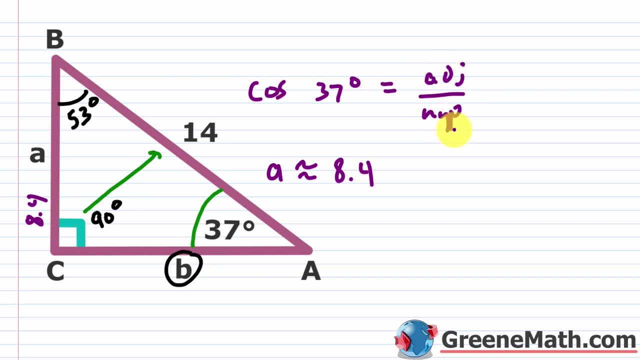 the adjacent over the hypotenuse, and the adjacent is what It's going to be. this lowercase b and the hypotenuse is 14.. Okay, so same deal. Very easy to solve this. Multiply both sides by 14,. 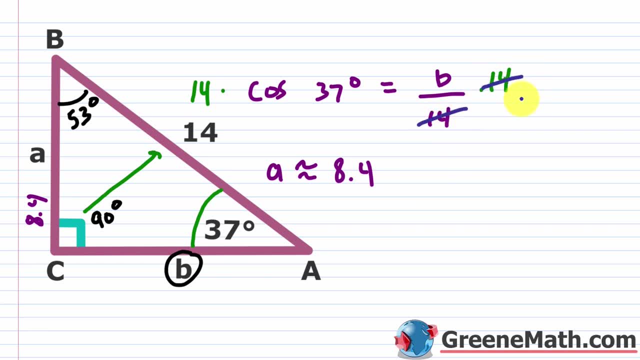 and what are we going to get? Well, we know that this would cancel with this and 14 times the cosine of 37 degrees. again, if you're rounding to the nearest tenth, you're going to get about 11.2.. Okay, so let's just say that b here I'm going to put 11.2.. 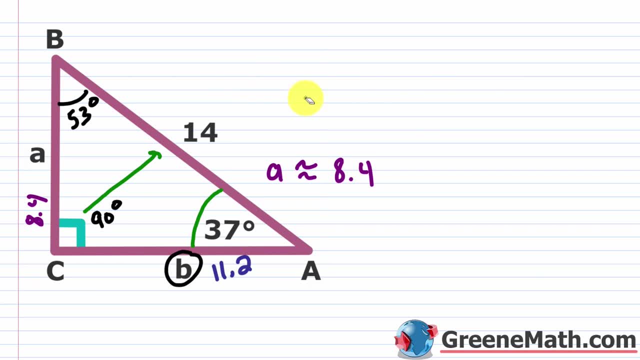 Again, we know this is an approximation, It's not an exact value, So we're going to put that b is approximately 11.2.. So we've solved this triangle, Okay. we have a value of 8.4 and a. 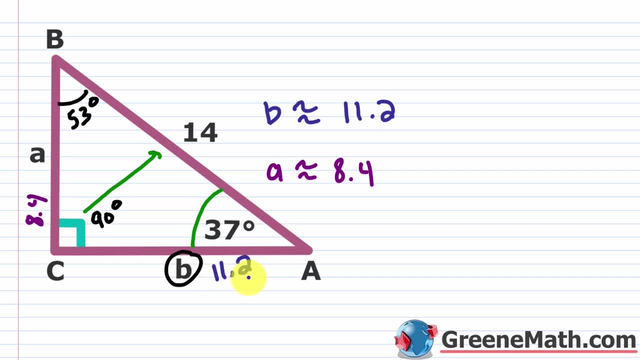 value of 11.2.. So we're going to put that b is approximately 11.2.. So we've solved this triangle: 11.2 for those two unknown sides. Again, those are approximations. You've got your 14,. 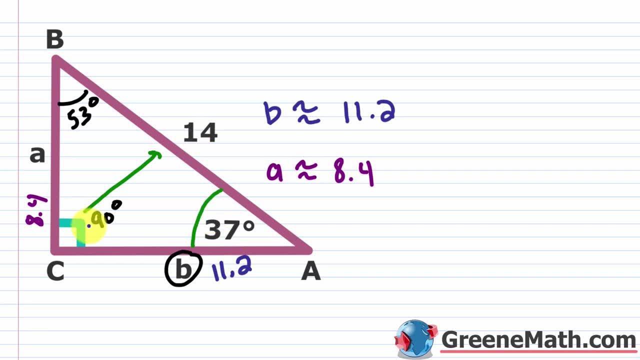 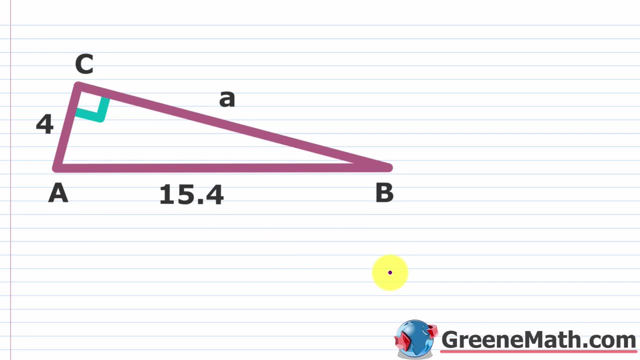 which was given- You've got this angle- is 37 degrees, which was given. We know this is 90 degrees, that was given. And then this guy we figured out was 53 degrees, All right, so let's look at a different type of problem. Now. we're solving a right triangle, but we're given two. 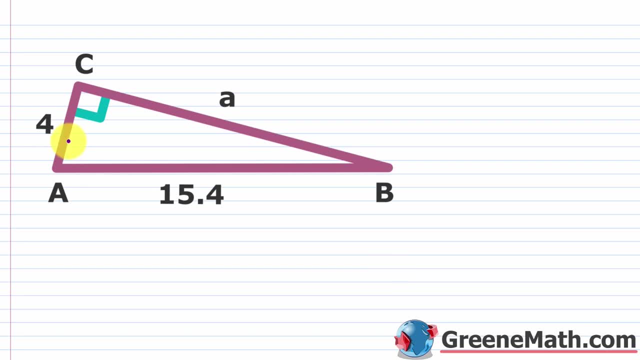 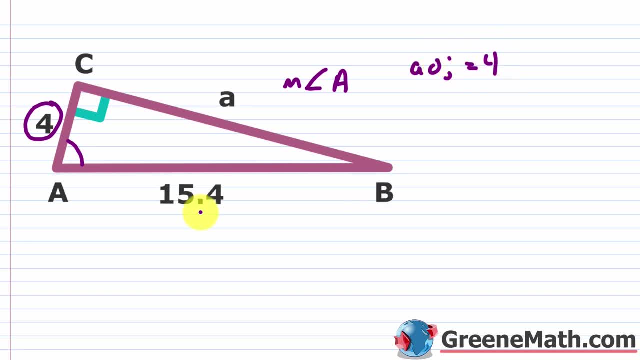 adjacent side. Let me just write that down. This is equal to 4.. We're also given the hypotenuse. Remember this is always across from the right angle. So we're also given the hypotenuse. This is 15.4 here. Okay, so what trigonometric ratio is the adjacent over the hypotenuse? It's cosine. 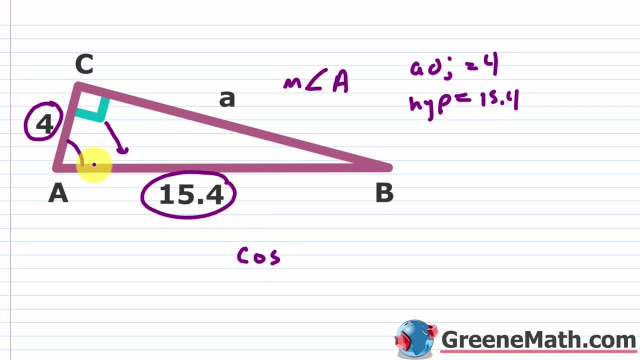 right, the cosine function. So we can go ahead and say that cosine of this angle a is going to be equal to. we would have the adjacent, which is 4, over the hypotenuse, which is 15.4.. Remember, we're not done here. Okay, we need to solve for a, which is our angle measure. 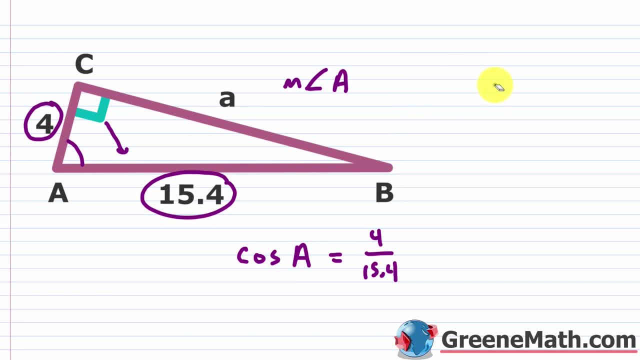 How can we do this? We talked about in the last lesson the fact that you could use the inverse of cosine- okay- to figure out what the measure of this angle was. In other words, I'm going to take my inverse cosine function and I'm going to plug this guy in. okay, the ratio in, So 4 over. 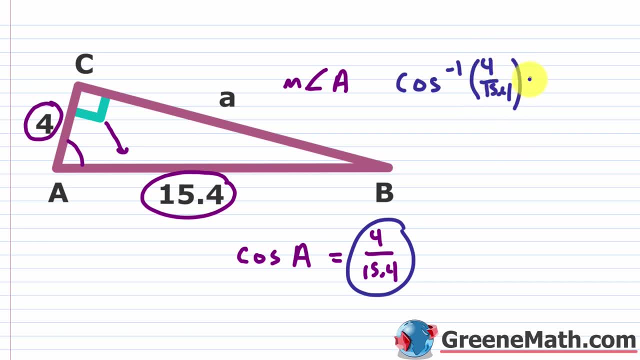 15.4.. And what I'm going to get out of this is going to be a value, that's a measure of my angle, a okay, and it's going to be approximated, I'm going to do, to the nearest 10.. So if you punch this up on a calculator and you round to the nearest 10th, you're going to. 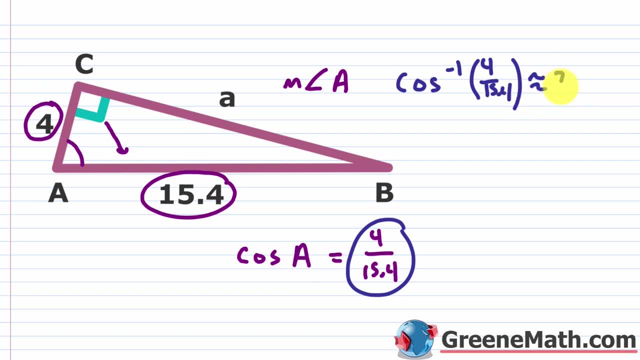 get about 74.9.. So let's just say this is about 74.9.. Okay, and this is going to be in terms of degrees. So let me put that there And let me just erase this. we don't need this anymore. I'm going. 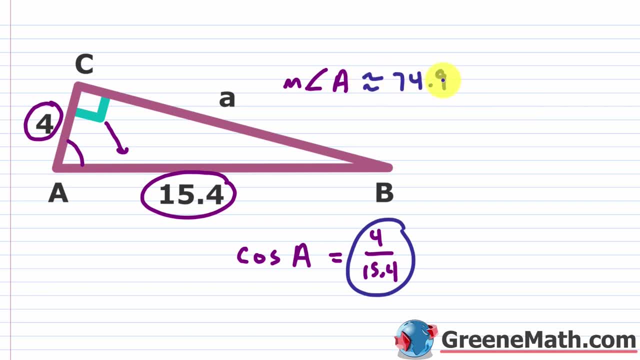 to say that this is approximately 74.9.. Okay, in here I'm just going to label this and say: this is 74.9 degrees. Again, this is an approximation, So let me put my degree symbol there And then let me label this. 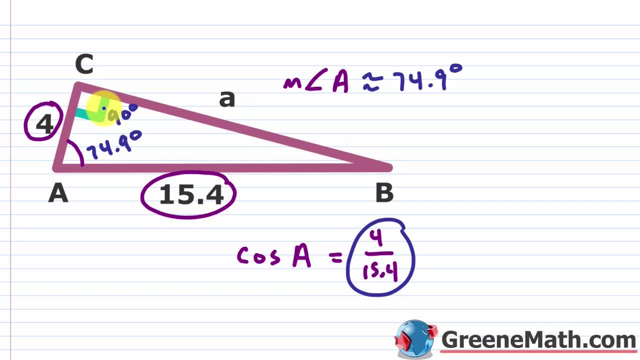 as 90 degrees. we already know that because of the right angle symbol. Now, what's going to be the measure of this? Again, this is just an approximation, But essentially we know that all three angles here would sum to 180 degrees, or the measure of angle a plus the measure of angle. 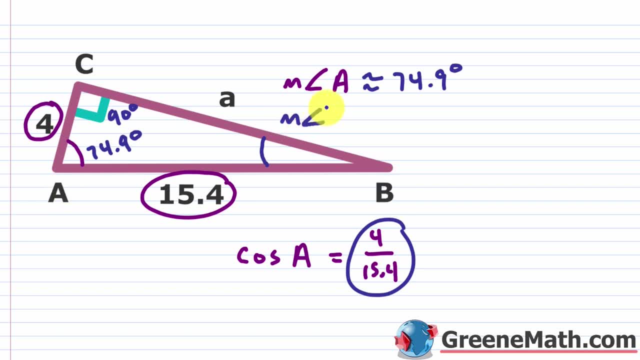 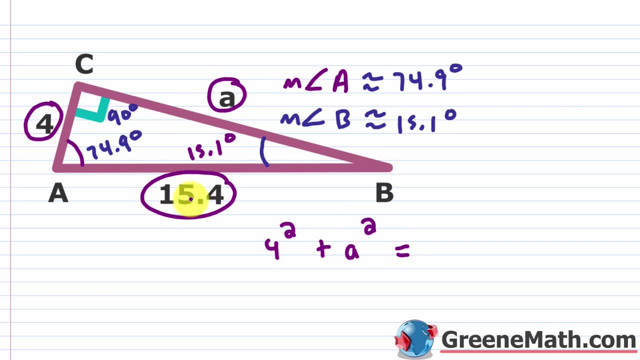 that's going to be a. that guy, squared is equal to the length of the hypotenuse, which is 15.4 squared. Okay, Now again, you're going to be estimating this. So four squared is 16.. Then plus a squared equals 15.4.. If I square that, I'm going to get 237.26.. So let me erase this. we're going to be solving for a, So I'm going to subtract 16 away from each side of the equation. Let me scroll down, I'll come back up. So. 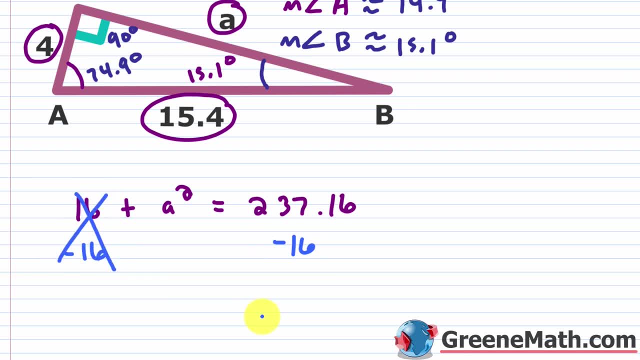 minus 16 over here. minus 16 over here. this is going to cancel. So you're going to have your. a squared is equal to: if I subtract away 16 over here, I get 221.16.. Let me erase this And let me just drag this up So we have enough room to work. Let's move this up here. And so what I want to do now is solve for a. Now, normally you would say a equals plus or minus the square root of this guy, right? But you don't need the minus here. you see the principal square root. So a is going to equal the principal. 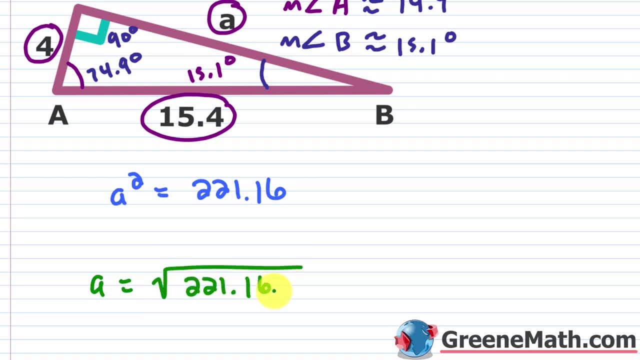 square root root of 221.16.. So that's approximately going to be 14.9.. Okay, Approximately going to be 14.9.. So let me scroll back up and we'll write this as our answer. I'm just going to put 14.9 here, So. 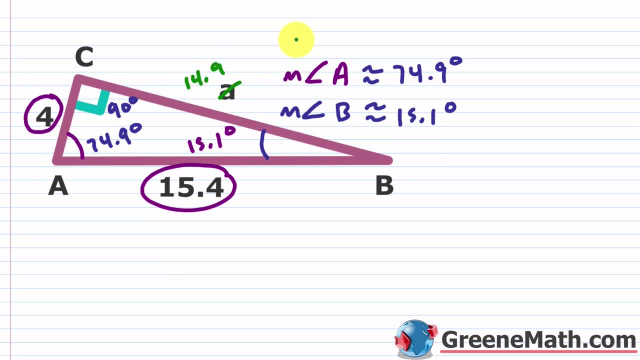 14.9.. And just to make sure everyone knows it's an approximation, I'll say A is approximately going to be 14.9.. Okay, In some of these problems you're going to have units. you might get inches or yards or feet or whatever you're working with. Just make sure you include your units. 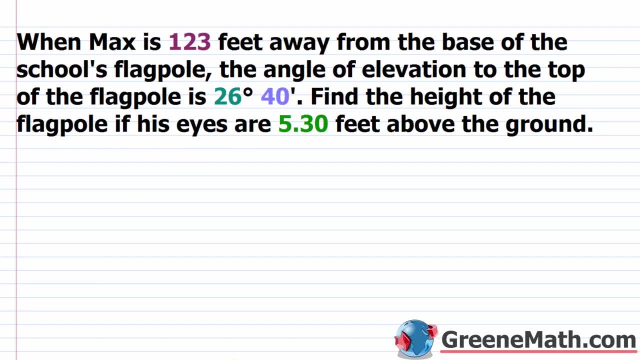 In this case we're not given any. All right, Let's look at a little word problem now. So when Max is 123 feet away from the base of the school's flagpole, the angle of elevation to the top of the flagpole is 26 degrees 40 minutes. We want to find the height of the flagpole. 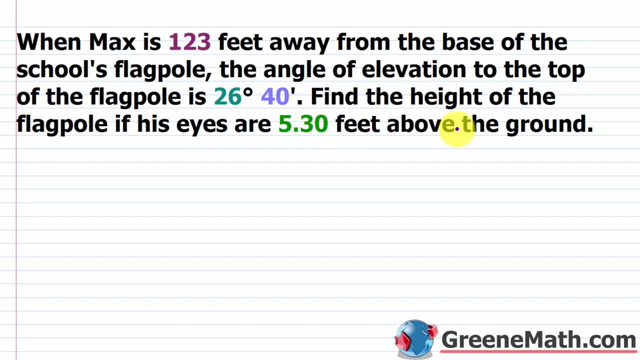 if his eyes are 5.30 feet above the ground. So when you first see problems that involve the angle of the flagpole, you want to find the height of the flagpole. So when you first see problems that involve the angle of the flagpole, you want to find the height of the flagpole. 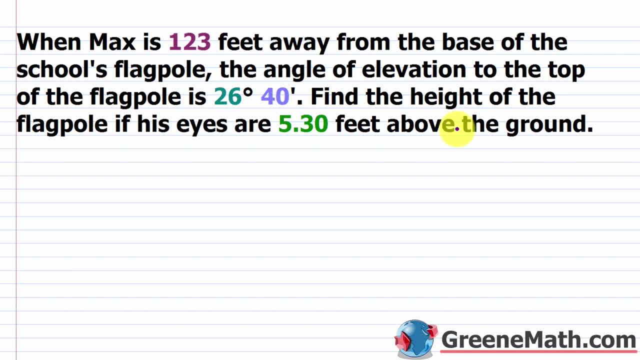 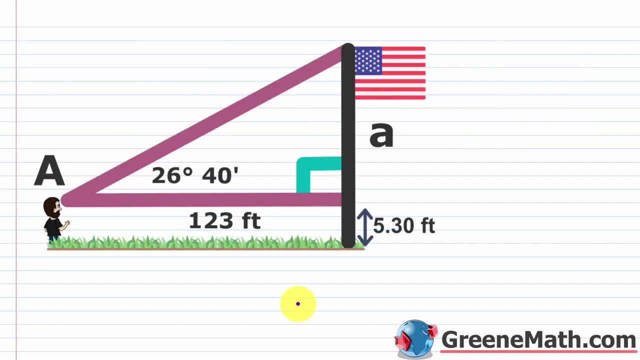 So when you first see problems that involve the angle of elevation or the angle of depression, it's a little bit confusing. What you want to do to clarify things is always draw a little picture. Okay, So that's what I've done here, And so basically you can see that this part right here. 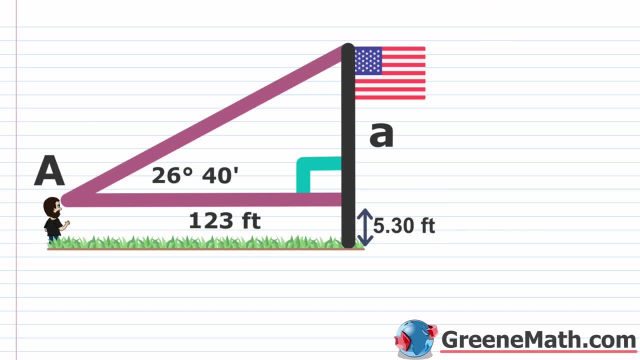 remember, his eyes are 5.30 feet above the ground. So 5.30 feet above the ground. So that's what this part is right here. If you think about this entire thing, okay, let me change the color here. This is what we're looking for: This height going all the way up to the top of the flagpole. 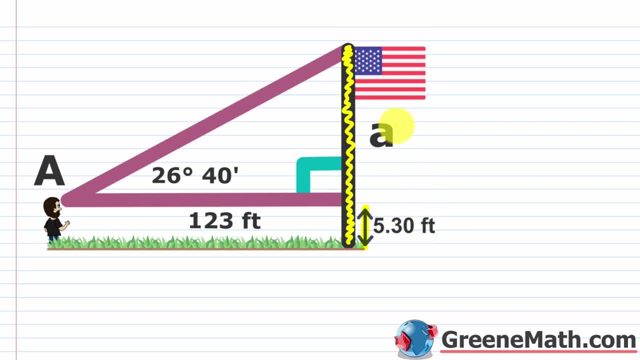 All the way down. So it includes this 5.30 feet plus the measure of this side A. Okay, So we need both of those. We need to add them together, Okay. So what we're going to do is we're going. 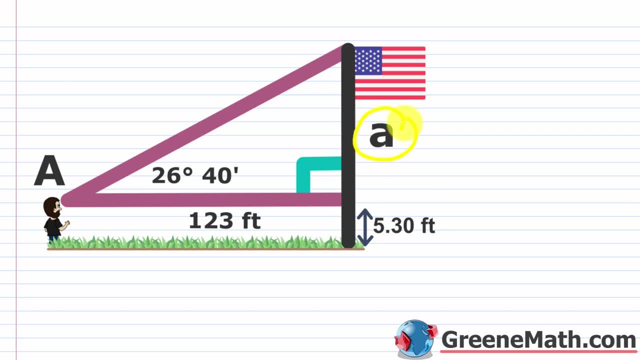 to work on this part first. So how can I find this unknown side A? Well, I'm given this angle measure here, which is 26 degrees, 40 minutes, Okay. So if I know that I have this guy right here, which is the adjacent side, Okay, And I want to find this part right here, which is the opposite. 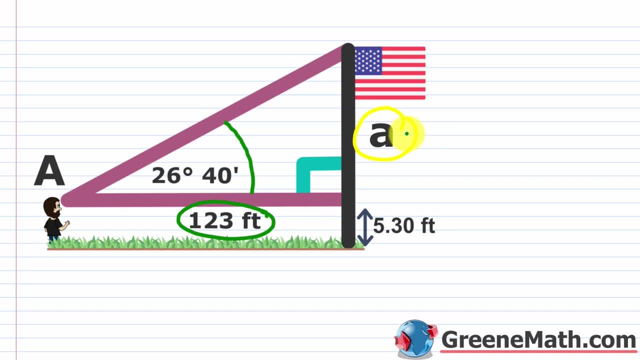 side. Well, which trigonometric ratio gives me opposite over adjacent? Well, I can use my tangent function, right? So I can say that the tangent, the tangent of this 26 degrees 40 minutes, is equal to the opposite side over my adjacent side, which is 123 feet. Okay, I'm just going to put 123, just. 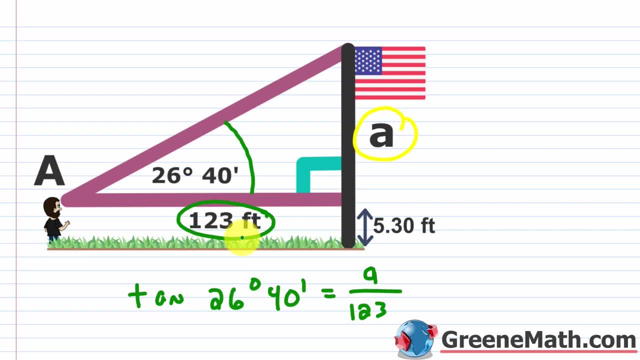 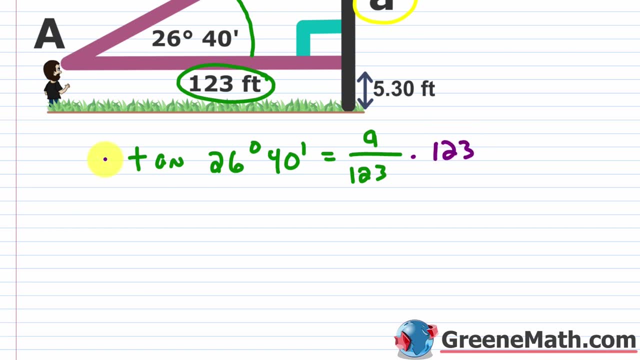 to work with the numbers for right now. Okay, So what we want to do is just multiply both sides by 123.. Let me scroll down and get some room going, So I'm going to multiply this side by 123 and this side by 123.. We know that this 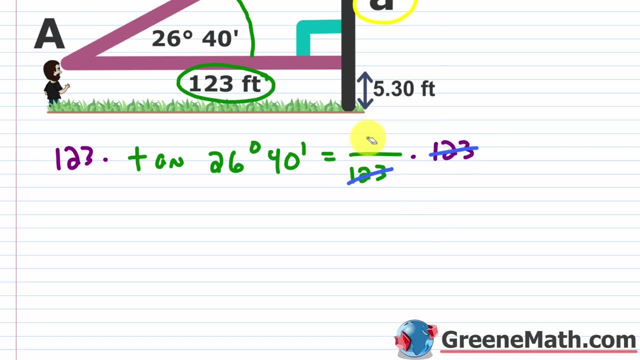 cancels with this and I'm left with just A Okay, And it kind of looks like a nine. So let me make that a more clear. So I would say that I'm just going to flip this over and say A is equal to. 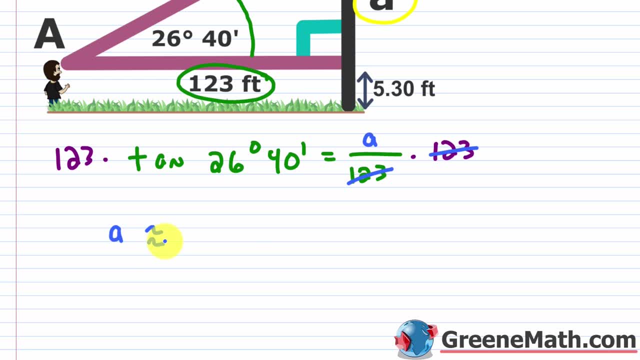 or actually, let's put approximately, because we're going to have to estimate this: If I did 123 times the tangent of 26 degrees 40 minutes, I would get about 61.8 feet. So about 61.8 feet, Okay Now, and I could just put FT to abbreviate that Now. 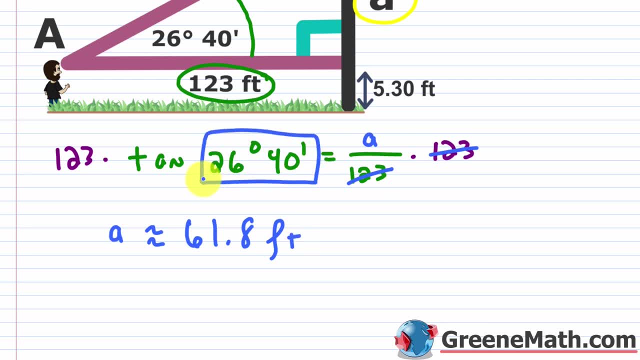 if you're confused about how to enter this into your calculator. you have on a TI-83 or 84, whatever you're using. you can hit second and then angle, Okay, And you can choose degrees and you can choose minutes- Okay, That way you don't have to convert it into a decimal. 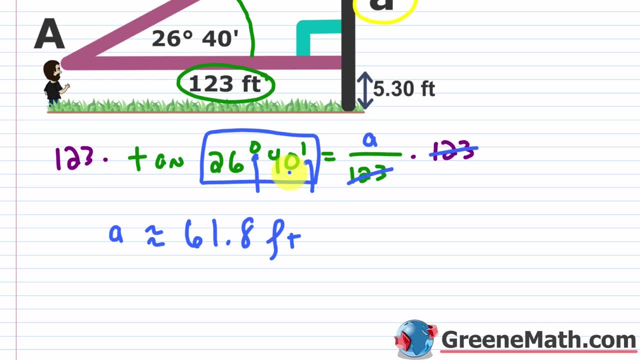 and then type it in. It's a little bit easier and it'll be a little bit more accurate. All right, So A is approximately 61.8 feet. Now we are not done. We haven't solved the problem yet. Let me erase all this. 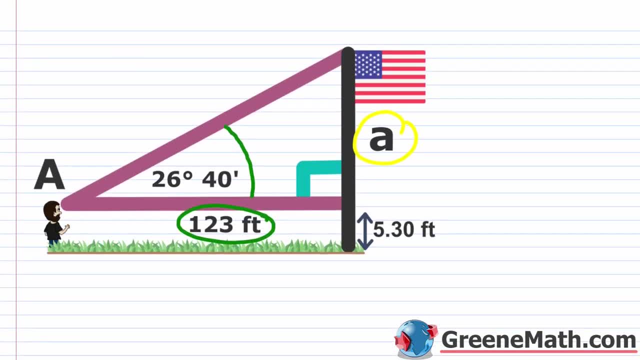 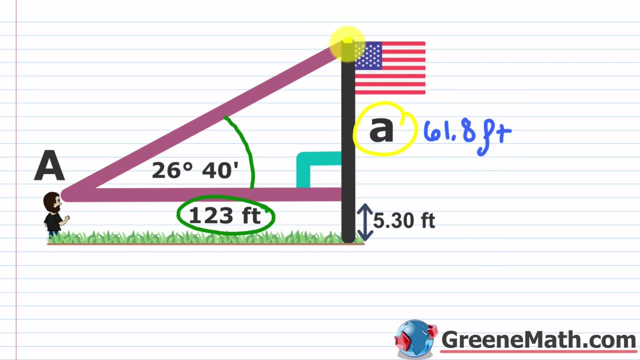 and let's go back up And let's say that this guy is 61.8 feet, But again, I'm trying to find the height of the flagpole, which goes all the way down. Okay, Remember, his eyes are 5.3 feet. 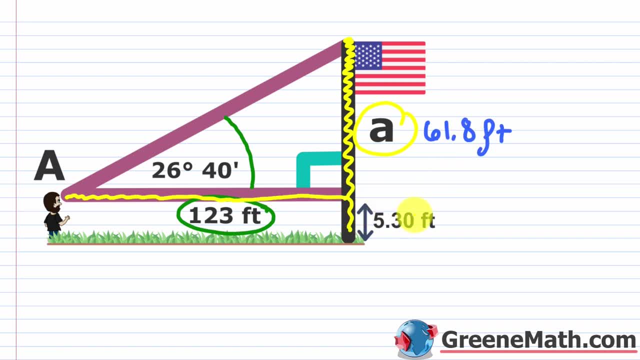 above the ground. Okay, So I've got to add these two guys together to get my final answer. So we're going to do 61.8 feet plus 5.3.. Okay, And this would give me- this would give me- 67.1 feet In this lesson. we want to talk. 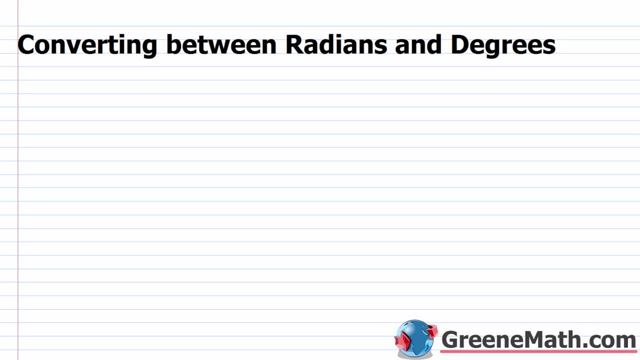 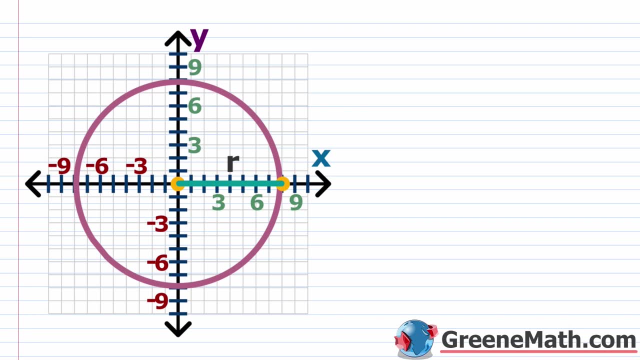 about converting between radians and degrees. So far in our course we have strictly measured our angles using degrees. Now, as we progress through this course and math in general, it's going to be more useful to measure angles using radians instead of degrees. This is going 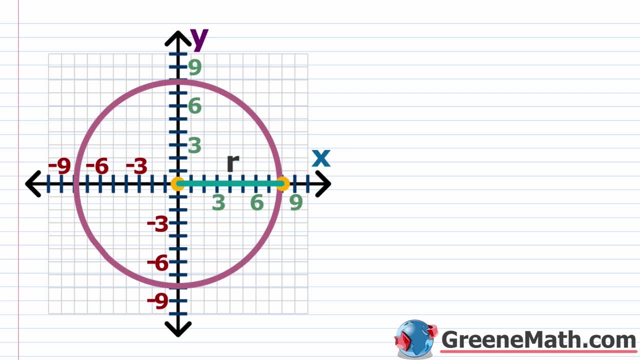 to allow us to treat trigonometric functions as functions with domains of real numbers. So what exactly is a radian? Well, a radian is going to be based on the radius of a circle. So I want you guys to recall that the distance from the center of a circle to any point on 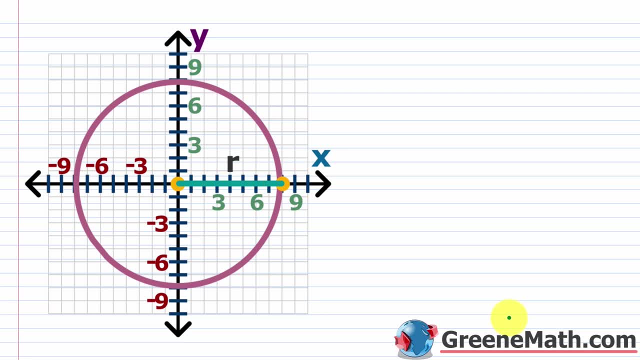 the circle is known as the radius, So typically we will denote this with a lowercase r. So let's look at this little graph we have here. We have a circle that's already drawn. I have made a point at the center of the circle and I have made a point just somewhere on. 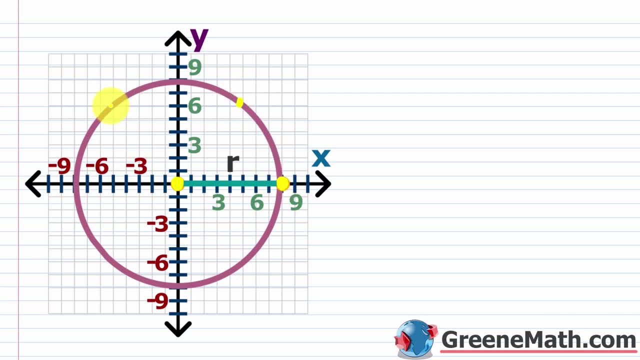 the circle. Okay, it's right here, but it could have been right here. it could have been right here, Anywhere on the circle. if I draw a line segment from the center to some point on that circle, the distance is always going to be the same. It's represented with that. 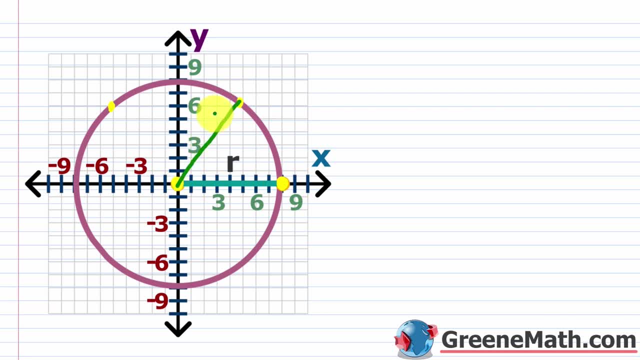 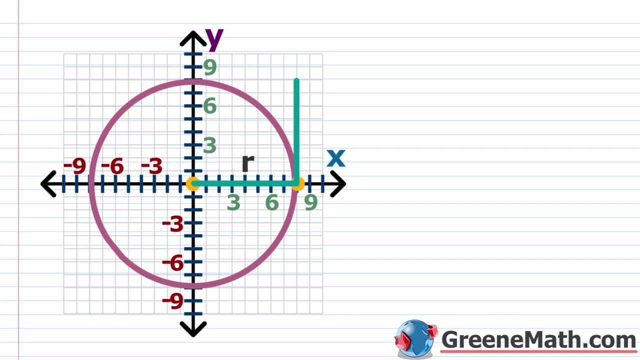 lowercase r. So if I drew this guy right here, this would have a distance of r. or if I drew this guy right here, this would have a distance of r as well. So let's say that we make a copy of our radius and we just 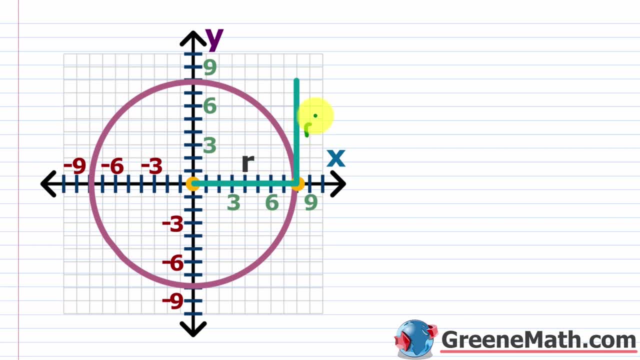 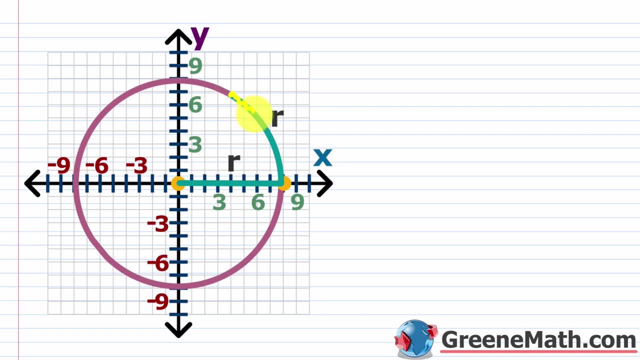 extend this vertically. So we'd say that this has a distance of r. and now let's bend this onto our circle again. to where? from right here, okay, starting right here, going all the way down to this point. and from right here going to this point. here, those both have a distance of r. So we understand what. 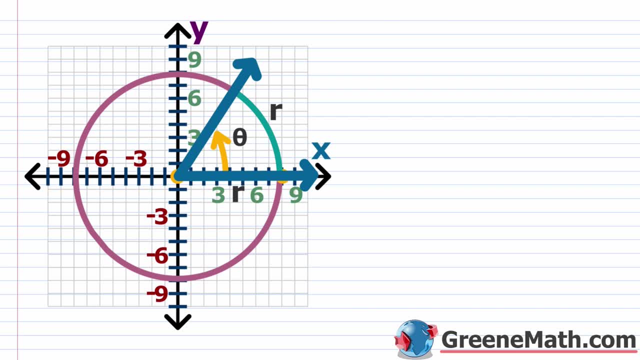 we're looking at here. Now let's suppose that we have an angle where the vertex is at the center of the circle and it intercepts an arc on the circle that's equal in length to the radius of the circle. So you can see, that's the exact situation we have here. We have the center. 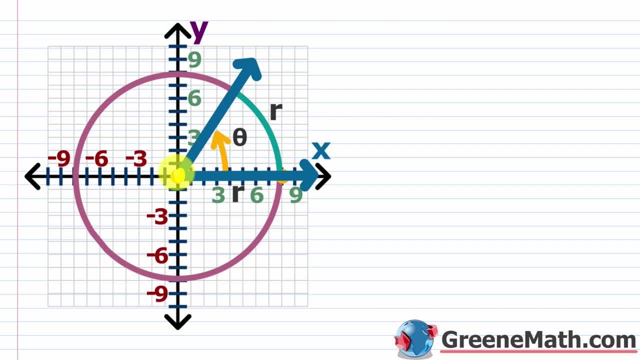 of the circle. that's the vertex of our angle and it intercepts an arc. okay, it intercepts an arc that is exactly equal in length to the radius of the circle. So when this case occurs, we can say that our angle theta is exactly equal to one radian. So one radian. Now let's extend this concept to two radians. 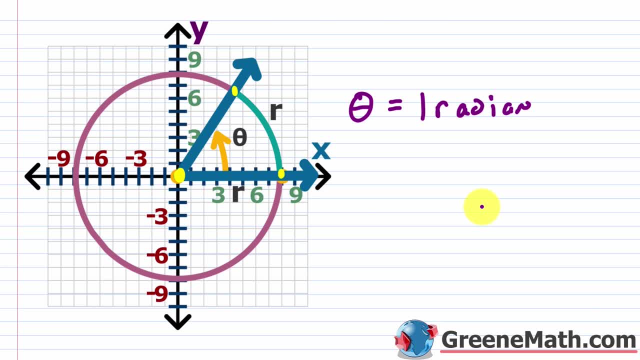 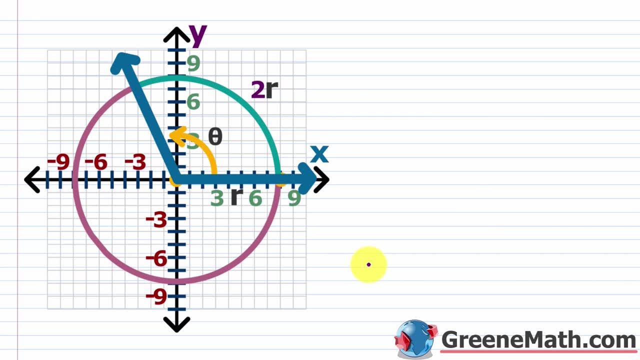 What would an angle of measure of two radians look like? Well, we have this here. So now you can see that the angle would intercept an arc that's equal to twice the radius of the circle. This is two times r, right. so from right here, from right here to right, here is r, okay, the radius This is. 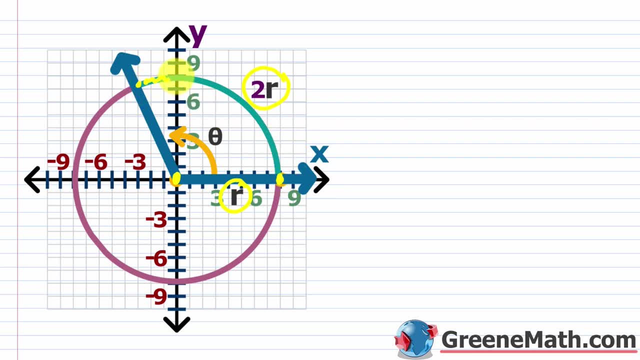 twice the radius of the circle. So we have this here, So now we have this here. So we have this two times r. so from right here to right here, okay, and I can highlight this in- So this is two times the radius. So in this particular case, we can say that theta is equal to two radians. okay, two. 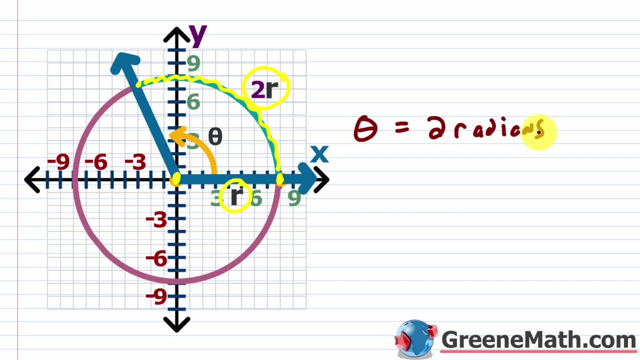 radians, So on and so forth. You can extend this concept and say: if the angle would intercept an arc that's equal to half of the radius of the circle, well then theta would be half of a radian Again, so on and so forth. So let's talk a little bit about how we can. 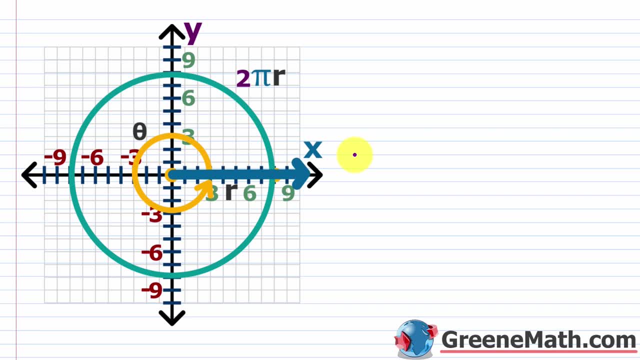 get a formula going to convert between degrees and radians. So in general, if our angle, theta, is a central angle of a circle of radius r- okay- and theta intercepts an arc of length s- then we can obtain our radian measure of theta. by saying that theta is equal to, we would have s. 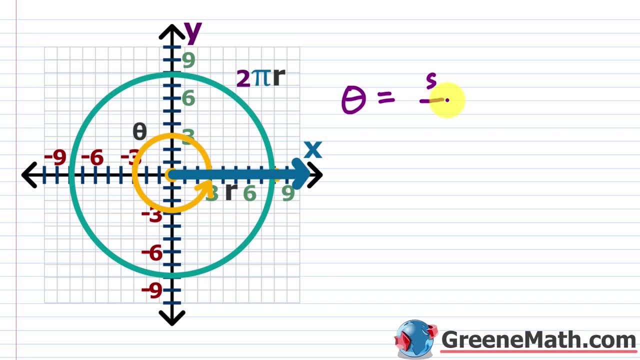 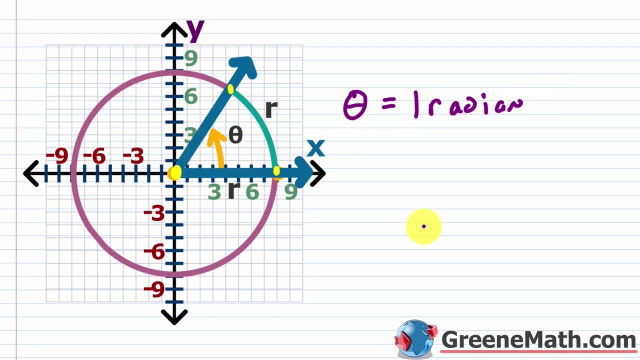 again, this is the length of our arc divided by r. this is going to be in terms of radians, okay, So if we go back to our circle of radius r, we can see that theta is equal to half of the radius of the circle of radius r. So if we go back to this example here, well, the length of the arc here is: 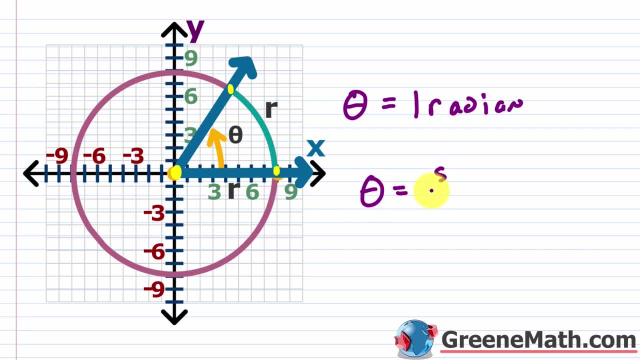 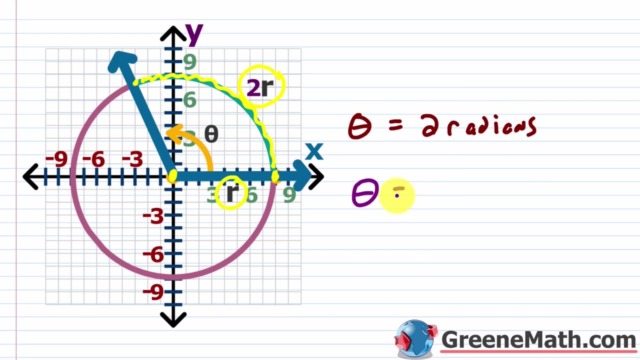 exactly r. So if we said theta is equal to s over r radians, well, now if I substitute in an r there, okay, you would have r over r, which is one, so you would get exactly one radian. If I come to this example here again, if you say theta is equal to s over r radians and I plugged in 2r there, so if I 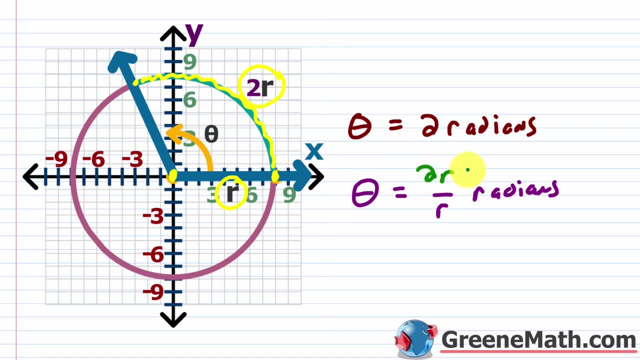 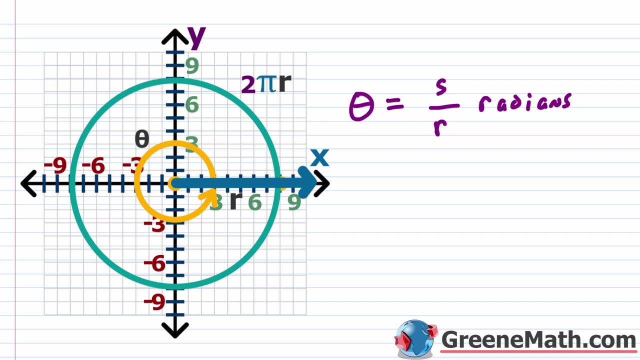 plugged in 2r here, so 2r. well, what's going to happen is the r's are going to cancel and you'd have two radians. So two radians. so that's where that comes from. So now let's think about this in terms of a 360 degree angle, and we'll use this to build a little conversion formula. So we know that. 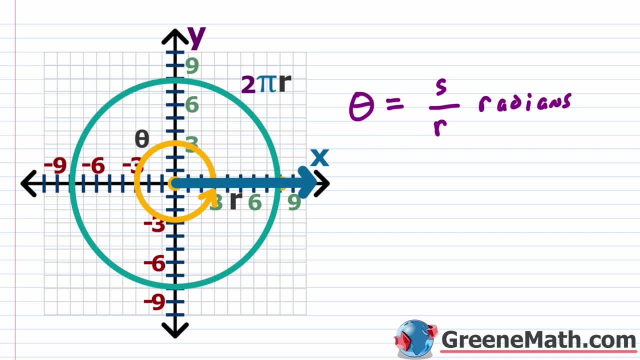 a 360 degree angle corresponds to one complete rotation or one complete circle. So I can just go over this. One complete rotation, okay. so we know that theta here is 360 degrees. okay, but in terms of radians, what is it? Well, let's think about the fact that the formula for the circumference of a circle, or 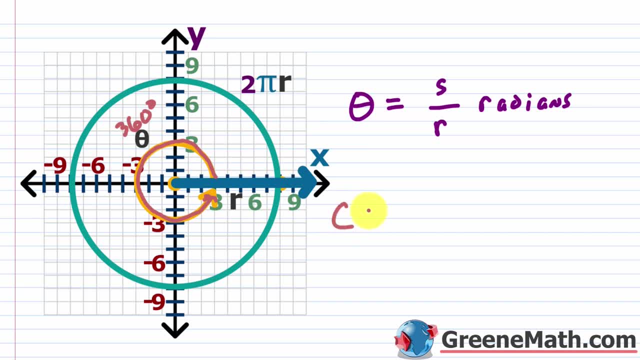 the distance around the circle c, for circumference, is equal to 2 times pi times r. Okay, so this is a formula you should know from basic geometry, if you don't, there it is. So, basically, if we think about the fact that a 360 degree angle corresponds to one complete rotation or one complete circle, 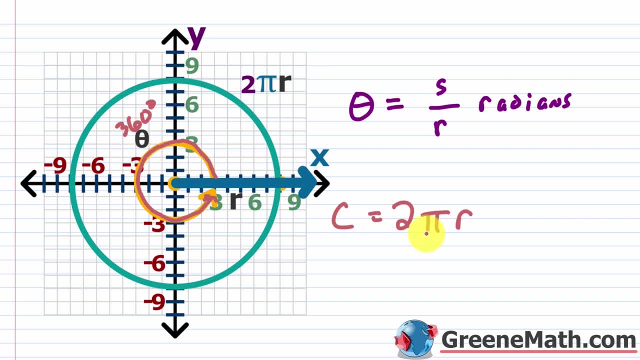 which again is one complete circle, intercepts an arc equal in length to 2 pi times the radius of the circle. Well, if I plug this guy in here, what do I get? Well, in this particular case, theta is equal to: we would have 2 times pi times r over r, this number of radians. So what's going to happen here? 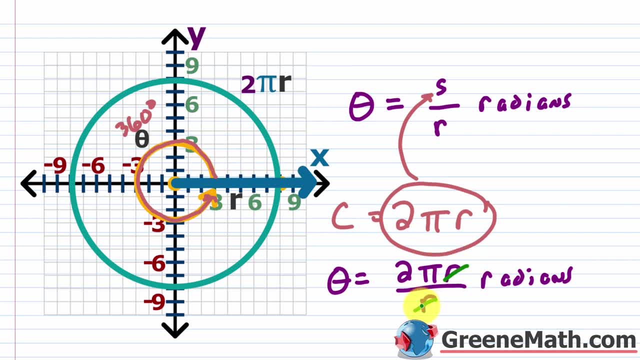 is that the radius and the radius. those are going to cancel from numerator and denominator. so that's gone and I'm left with 2 pi radians. Okay, so for a 360 degree angle it's 2 pi radians. So let's go ahead and erase this and put 360 degrees equals 2 pi radians. Okay, so we're all in agreement on that. 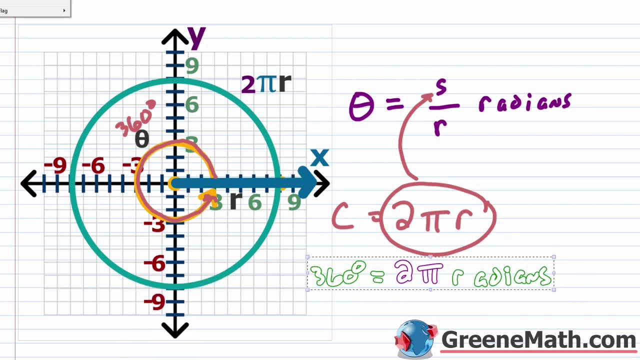 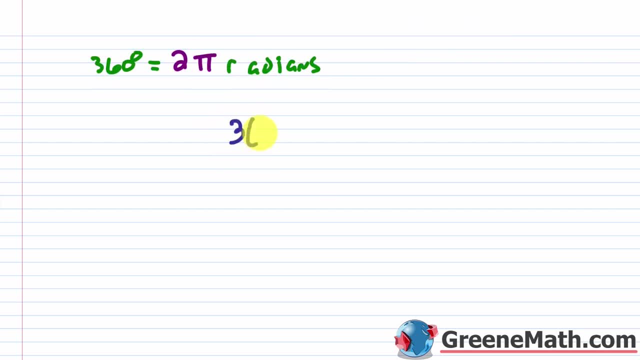 let me just copy this real quick and let's go to a fresh sheet. So let's paste this guy in here. I'll just drag this down here. let me just write this in a neater format. so 360 degrees is again equal to 2. 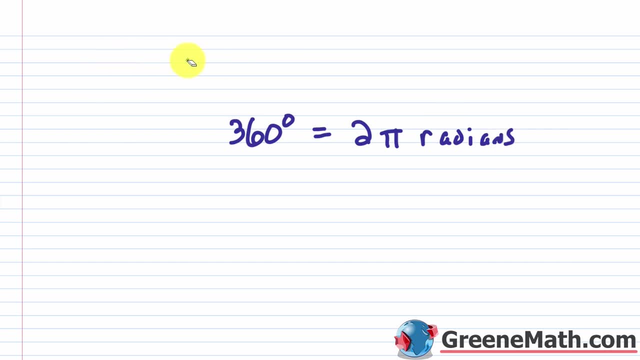 pi radians. Okay, all right. so what we're going to do now is actually divide this okay by 2 on each side. So if I divide this by 2 and this by 2, what I'm going to get half of a 360 degree angle, or. 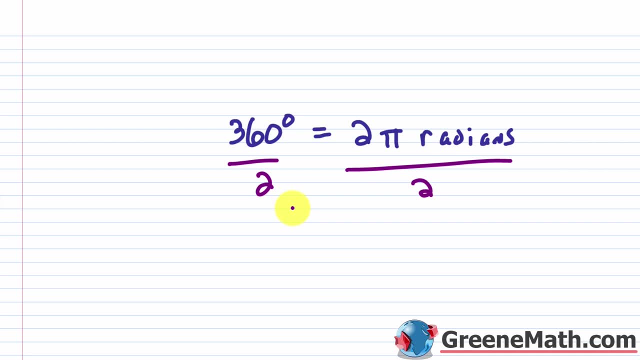 half of a full rotation is half a rotation, right, so it's 180 degree angle, or a straight angle. So we would have that 180 degrees is equal to the 2s would cancel there, right? so I would just have pi radians and this is the relationship that you're going to see in most of the equations. So let's. 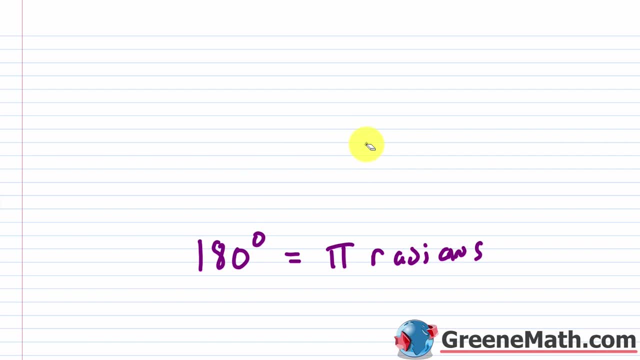 erase this real quick. and let's drag this up here, and I'm going to show you a few different ways. you can think about this Now, when you work with some type of conversion problem, generally you want to set up a fraction that's equal to 1, where what you want to end up with is in the numerator, So in 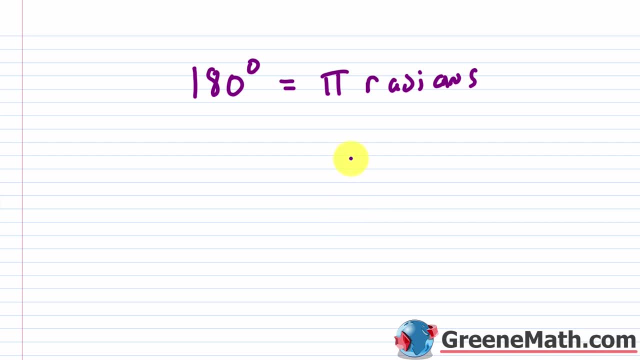 other words, for these problems, the way I would do it is I would say: okay, you can say 180 degrees over pi radians. okay, like this: If you're trying to convert to degrees, okay, or if you were trying to convert to radians, you could say that you had pi radians. 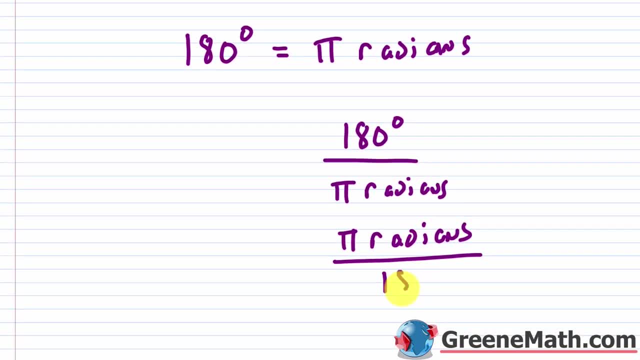 pi radians over 180 degrees. okay, So either of these would work. it's just a matter of what you're trying to cancel. Am I trying to cancel out degrees? Am I trying to cancel out radians? What you want to end up with needs to be in the numerator, so let's keep that in mind. 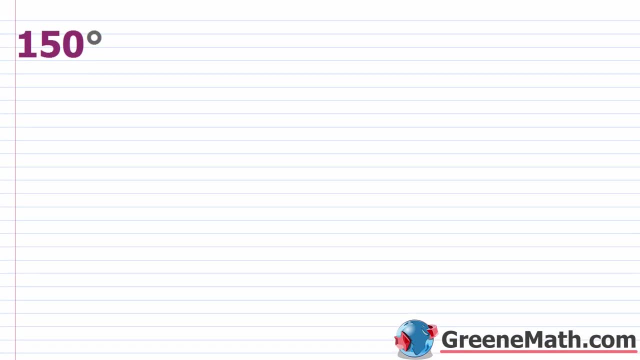 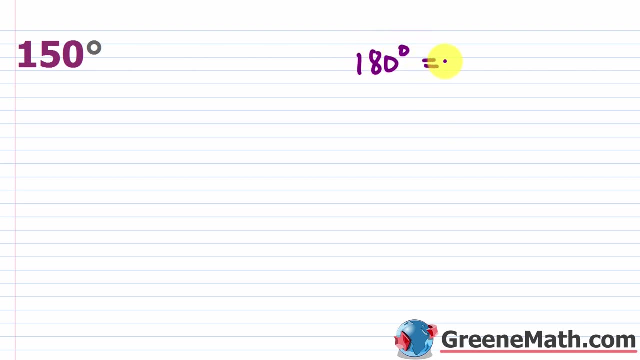 So let's go to the first problem here. and we have 150 degrees. So again, the relationship is that you have 180 degrees is equal to pi radians. So I'm just going to write that down. This is something you should memorize so that you always have that in your head. 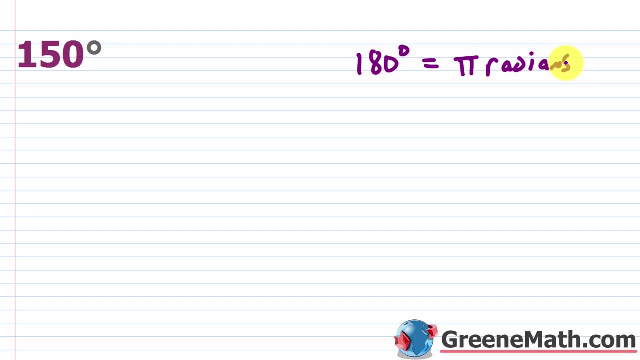 okay. So if I want to convert to radians, I want degrees in the denominator, okay, So what I'm going to do is I'm going to multiply this by pi radians- okay. pi radians over 180 degrees- okay, Let's erase this. we don't need this anymore, for right now. 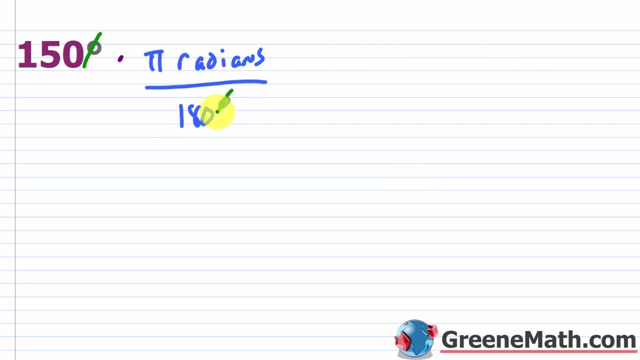 Let's just think about what's going to cancel. Well, degrees would cancel, so you can get rid of that, okay, and so we know our answer would be in terms of radians. and now I'm just going to go through and say, okay, well, 150 is divisible by 30, right? If I took 150 and divided by 30, I would be left. 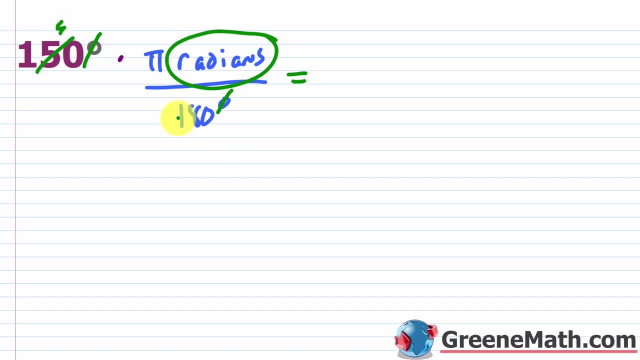 with exactly 5.. If I divided 180 by 30, I would be left with exactly 6.. So what I'm going to have is 5 times pi over 6 radians, So 5 pi over 6 radians. Okay, so very easy to convert these guys, and you can erase this right, just so you can show the. 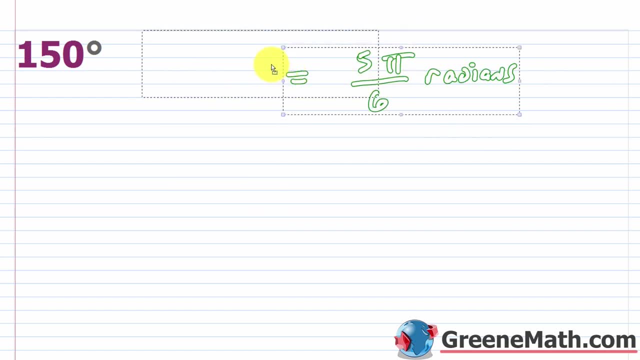 relationship. Let me just kind of scooch this over so we can make it nice and neat for our presentation. So 150 degrees is again equal to 5 pi over 6 radians. Let's look at another one. So we have 260 degrees Again. I'm just going to multiply this by 180 degrees is equal to pi. 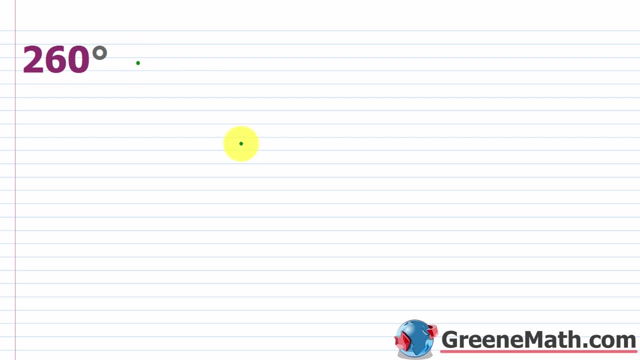 radians. So I want degrees in the denominator. so I want to get rid of that. So I'm going to say that pi radians Is going to go in the numerator and 180 degrees is going to go in the denominator. So I'm just going to cancel this with this. Those are gone and I would say that, okay, 260 and 180. 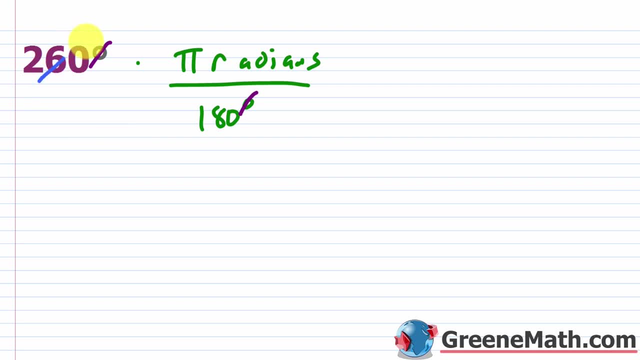 they're each divisible by 20.. Okay, so I can say that 260 divided by 20 is 13 and 180 divided by 20 is 9.. So this would be equal to 13 pi. okay, over 9, this number of radians. Okay, all right. so now. 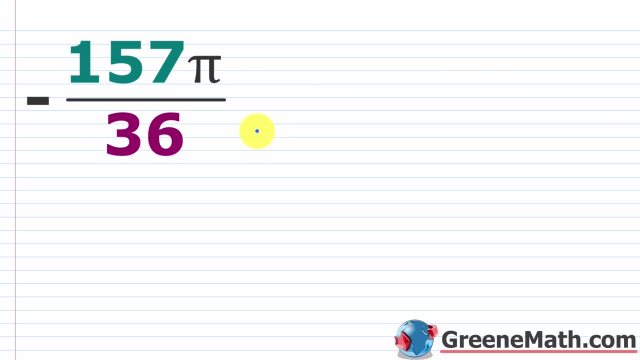 we have negative 157 pi Over 36. this is, of course, in terms of radians, So let me just go ahead and write that in real quick. So this is in terms of radians and we want to convert this into degrees. So again, I'm going. 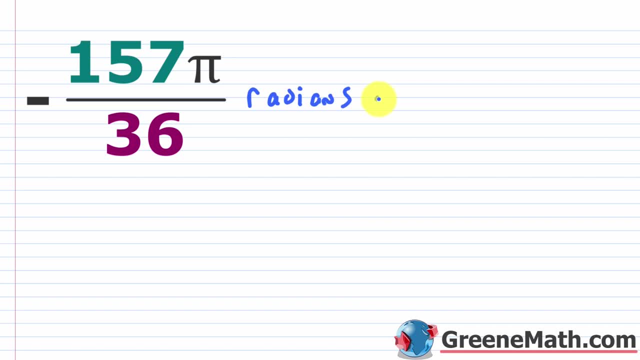 to multiply now. I would want radians to be in the denominator here and degrees to be in the numerator. So 180 degrees would go in the numerator and then we would put pi radians in the denominator Again. if you just remember this relationship: 180 degrees equals pi radians Again. 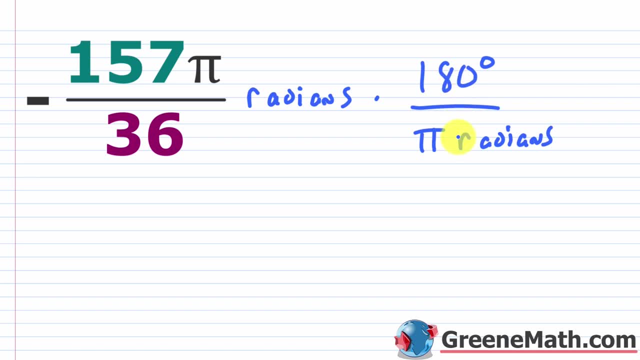 this is because these two guys are in the denominator. So I'm going to put pi radians in the denominator. So I'm going to put pi radians in the denominator Again. this is because these two guys are equal to each other. This fraction has a value of one. We're just using it to kind of cancel what we. 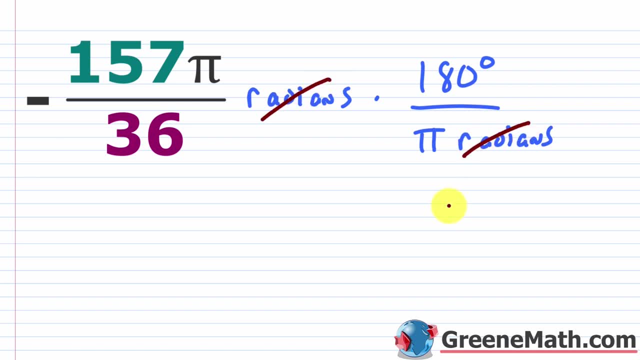 don't want, In this case, we don't want radians, So that's going to cancel. We're going to get rid of pi in each case, And so this is going to be equal to what? Well, you'd have 180 divided by 36, which? 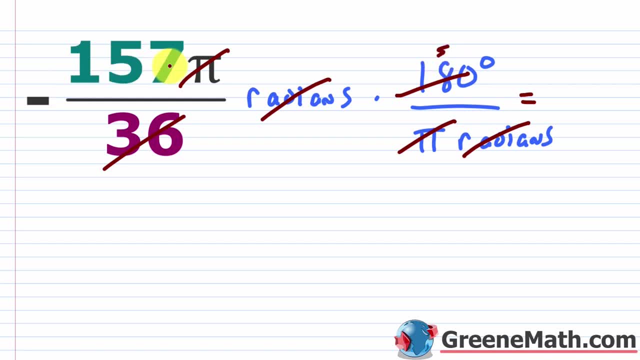 is going to give you 5.. So you have negative 157 times 5 degrees. So this would be negative 785 degrees Again. if you wanted to make this more presentable. if you're turning this in for a test or something like that, So you're going to put pi radians in the denominator. So this is going to 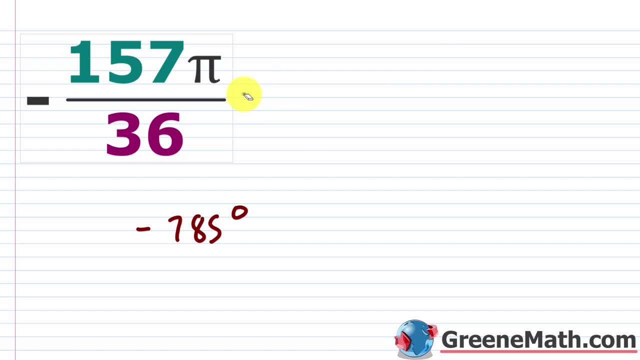 be like this, Then you can erase all that and just put- let me put radians in here to be clear- So radians and we'll put is equal to negative 785 degrees And I'll just erase this here. So negative 157 pi over 36 radians is equal to negative 785 degrees. Okay, let's do one more. Again, a very easy. 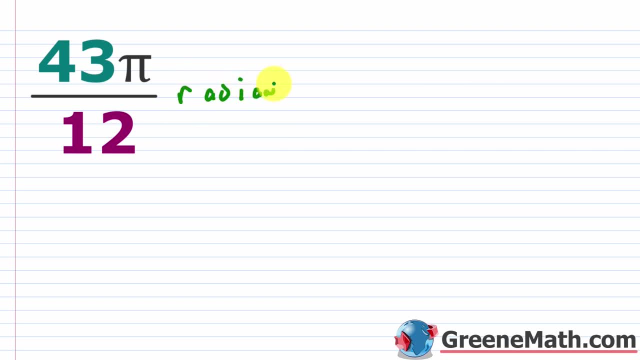 concept. I'm going to say this is in terms of radians. So 43 pi over 12 radians. I'm going to multiply this by what I want radians in the denominator. So I'm going to multiply this by the denominator. So I want 180 degrees in the numerator. Again, I want this in terms of degrees. 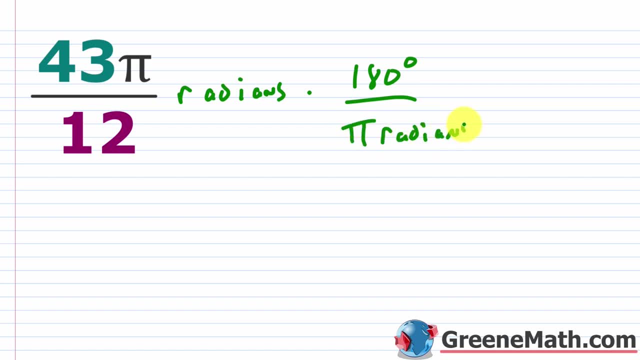 So I'm going to put pi radians in the denominator, And of course, this cancels, This cancels, And so what I end up with is what? 180 divided by 12 is going to be 15.. So this will be 15, and that'll be. 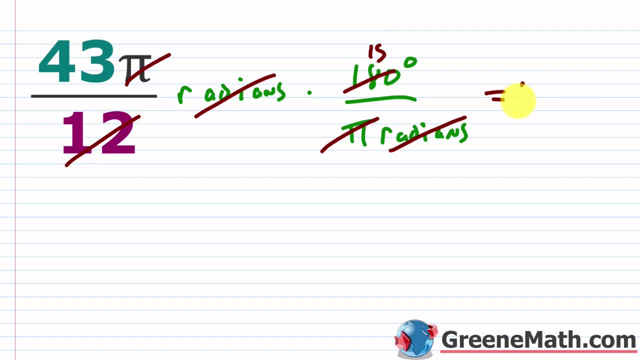 gone, And then 43 times 15 is 645.. So this would be 645 degrees Again. if you want to clean this up a little bit, you just erase all this. So I'm going to put pi radians in the denominator And. 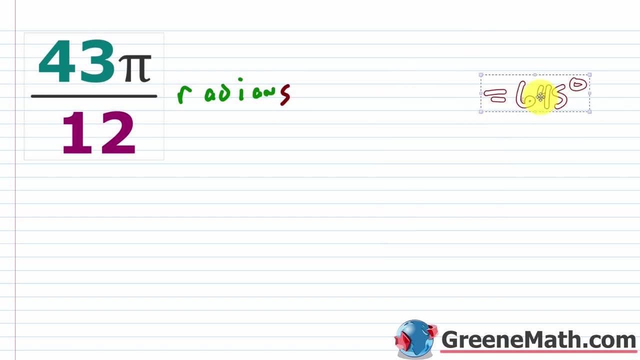 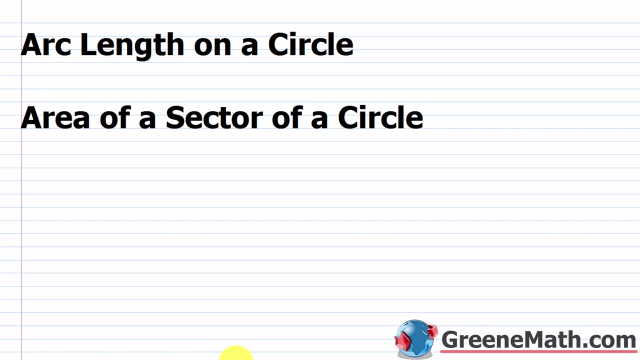 let me put this back and we'll just slide this over. We'll say that 43 pi over 12 radians is exactly equal to 645 degrees. In this lesson we want to talk about how to find the arc length on a circle, And also we'll look at how to find the area of a sector of a circle. All right, in the 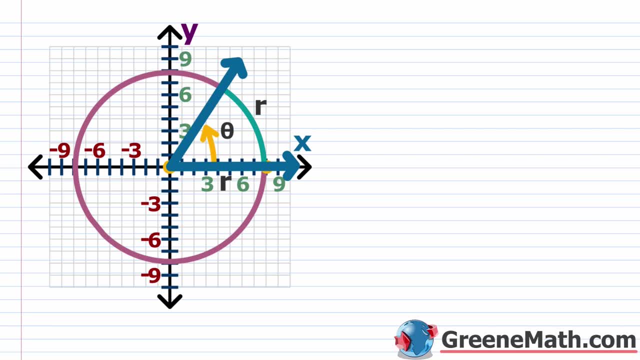 last lesson, we learned how to measure our angles using radians instead of degrees. So now what we're going to do is we're going to take our little formula. We're going to take our little formula And we're getting it a formula for finding the arc length on a circle. So let's recap what we 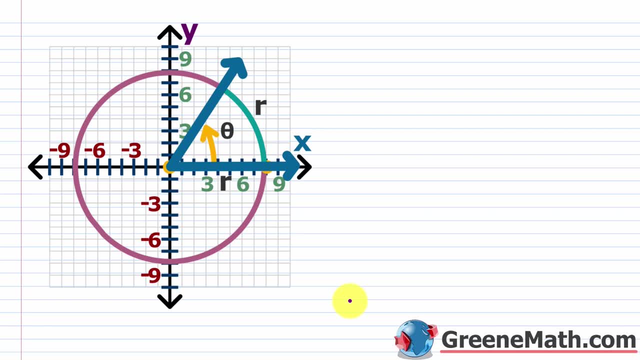 learned in the last lesson. So if our angle, theta, is a central angle of a circle of radius r And theta intercepts an arc of length s, Then we can obtain our radian measure of theta, as We say that theta is equal to s over r. Okay now, in this first example, what I've done is I've made this: 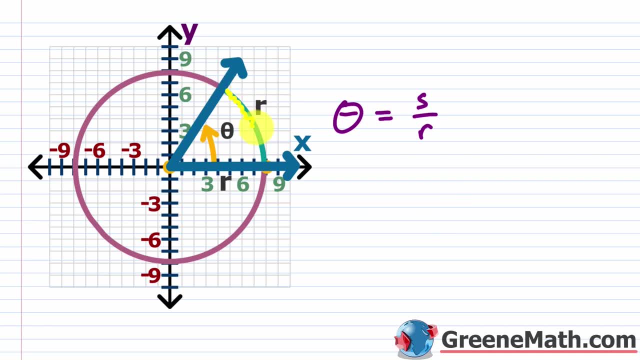 one available in c script. So when k is represented by v and v Quandt, The measure is going to be r over vm. But if I say theta is equal to s over vm, it can be different, And so we're going to. 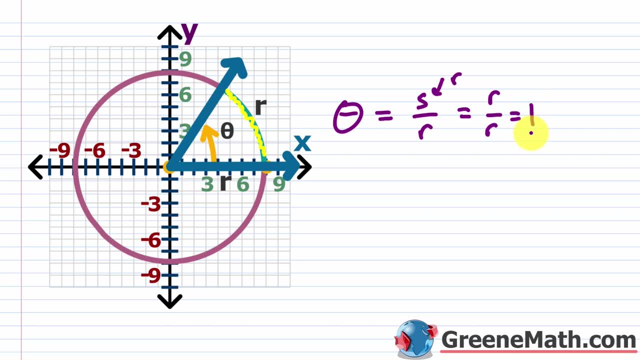 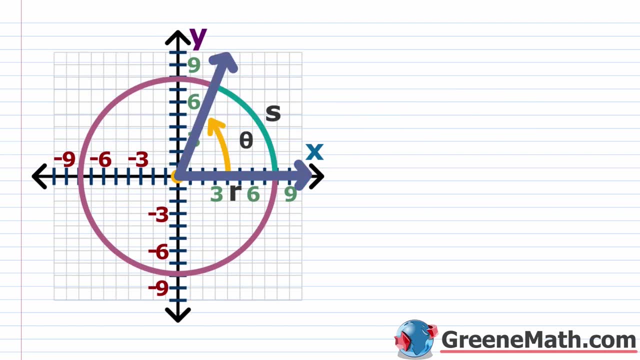 take that measure and combine it with our radius. This comes out. we see our radian value. It behind the c script. That will give us our gradient. Now if I enter the Всем Apostλη denominator and start calculating, the dud is I'm going to simply start manipulating the dumb. It'll institute the 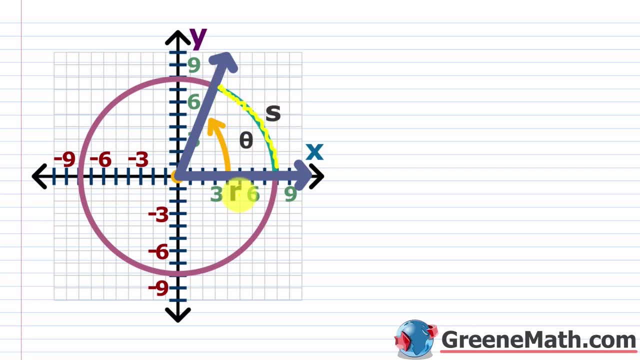 equation. So I have div. I'm going to substitute, I'm going to substitute this into a times theta going to just be represented with s. okay, so it's no longer equal to r. so in this case, we just go back to that little ratio and we say that theta is equal to s over r. okay, so s over r. but what? 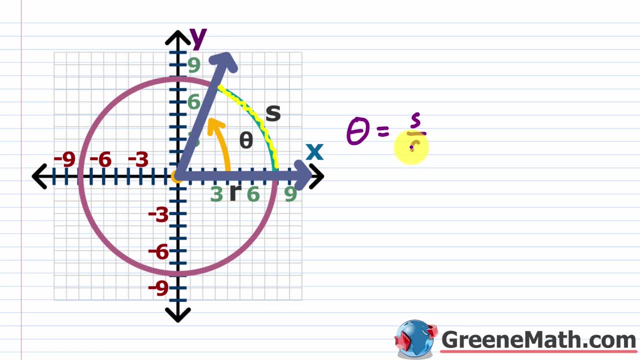 this is telling me is that I could rearrange this equation. okay, and I could solve for s. I could solve for s given the fact that I know the measure of my angle, theta, in radians, and I know r, which is the length of my radius. so what I do is just multiply both sides by r. okay, by r, and I'm going. 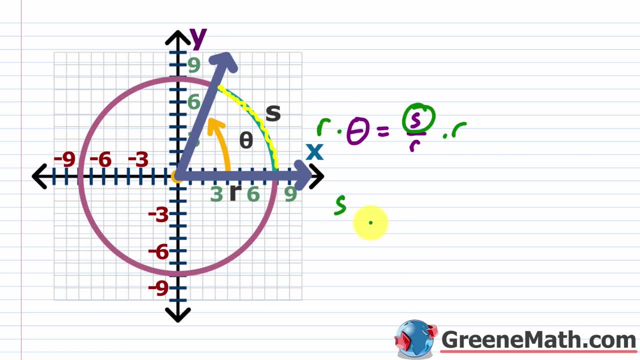 to get my formula, which is that s- again, that's, the length of the arc here- is going to be equal to this cancels, so I would have r times theta. okay, and theta has to be given in radians for this to work. if you get something in degrees, you just need to convert it, or you could use another formula. 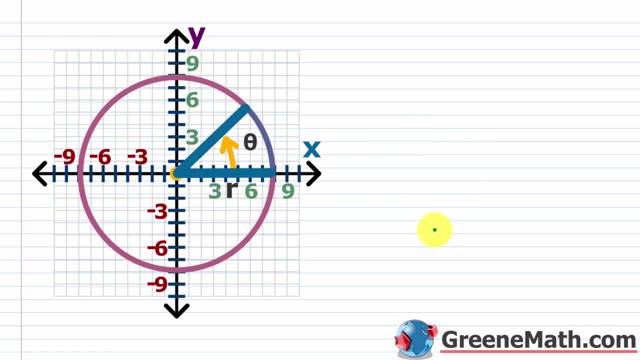 from geometry, which I'll cover in a little while. all right, let's go ahead and do that and see if ahead and take a look at an example. So we have an angle here which is marked as theta, and theta is going to be equal to, in terms of radians, pi over four. okay, and then we have our radius r. 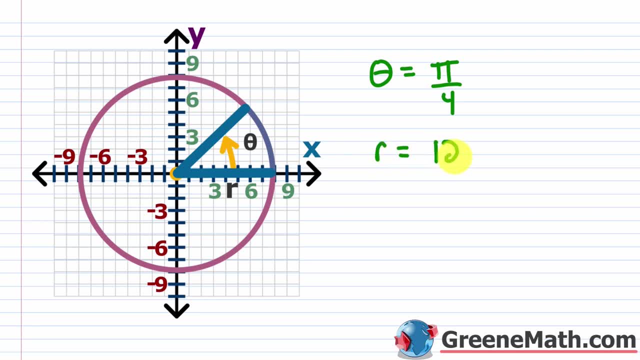 okay, so r is going to be equal to. we're going to have 12 miles here, so I'm just going to put mi to abbreviate miles. So what we want to do for this problem is find the length of this arc here. okay, find that length. So again, how do we do this? We're just going to use our little formula. 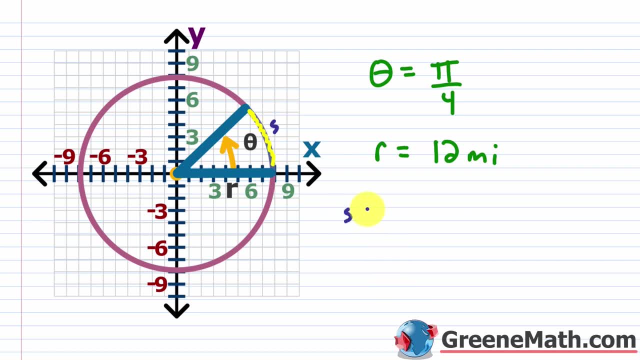 We're going to say that s- okay, I'll mark this with s- is equal to what It's equal to r, this radius measure, okay, which is 12 miles in this case, times theta, okay, and theta in this case is pi, pi over four, okay. So very, very simple math here. I'm going to cancel this 12 with this four and get 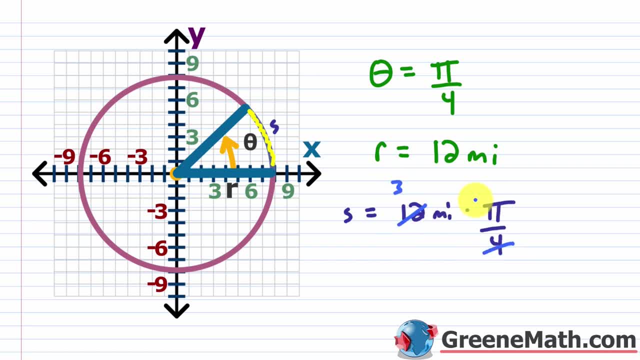 a three, and basically what I'd have here is three pi miles. okay, So s here is equal to three pi miles, and you could write out miles or you could put mi. it doesn't really matter. I think I'll just stay consistent and put mi there and leave it as. 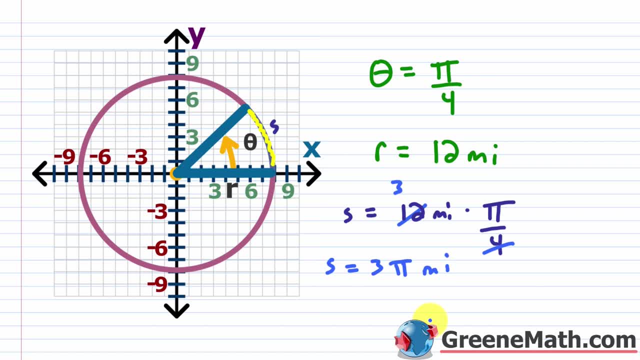 an abbreviated version. Now, depending on the context of the situation, you might want to give an exact answer like this, or you might want to punch up three times pi into a calculator and get an approximation and write it that way. It just depends on what your teacher's asking for. Okay, 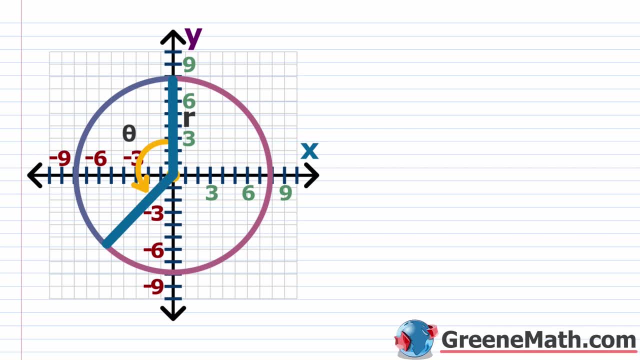 let's take a look at another example. So let's suppose that now our angle theta, our angle theta here, okay- is given as 135 degrees. Okay, so now we're working with degrees. and then r, the radius, let's say that this is 12 inches. So 12 inches Again. I'm just going to abbreviate that. 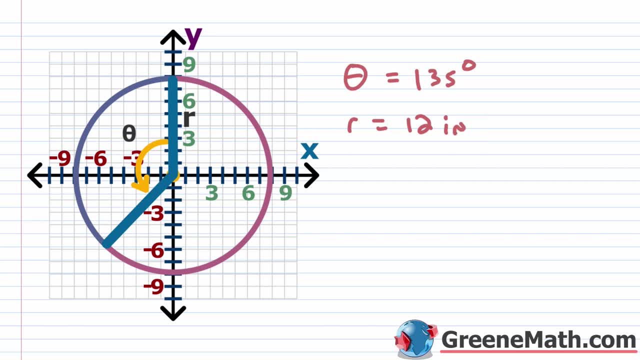 So what do we do here? Well, one strategy. if you want to use the formula that we just talked about, this into radians, So remember how to do that. Pi radians is exactly equal to 180 degrees, So I would say 135 degrees times. Remember how to do this. You want the units that you want to cancel. 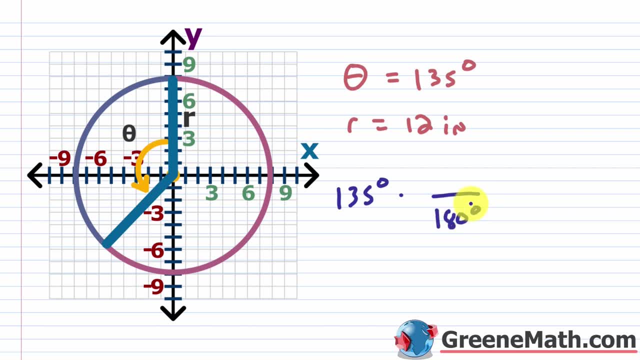 in the denominator. So I'm going to put 180 degrees down here and I'm going to put pi radians up here. You don't need to write radians, So I'm going to cancel this with this. So degrees are. 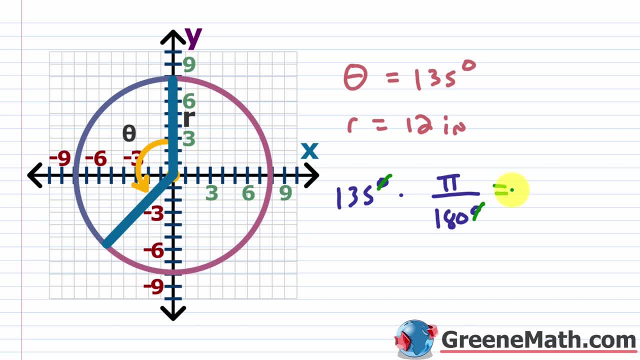 gone. So the answer I get here is going to be in terms of radians. now, okay, So let's think about 135 and 180.. What's going to be common between the two? Well, each would be divisible by 45.. 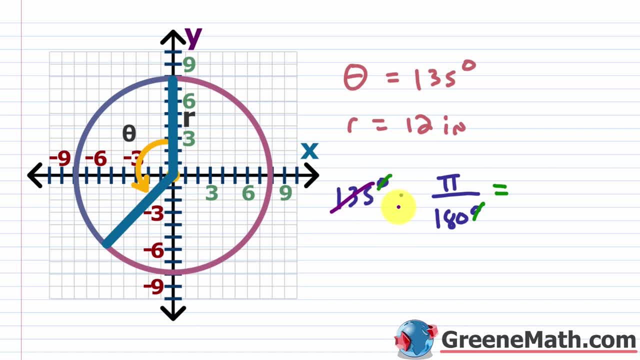 If I divided this guy by 45,, I would get exactly 3.. If I divided this guy by 45,, I would get exactly 4.. So this turns out to be 3 pi over 4 in terms of radians. okay, So. 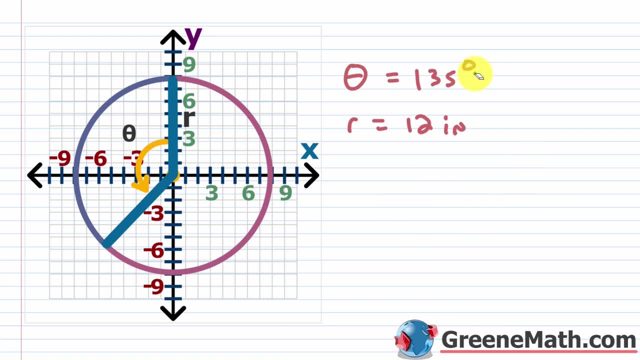 I'll just erase this real quick and I'm just going to erase 135 degrees and put 3 pi over 4 for radians, And now we're basically good to go. Again, we're trying to figure out what is the length of this guy. okay, And I'm just going to mark that and say that this is s okay, So s is. 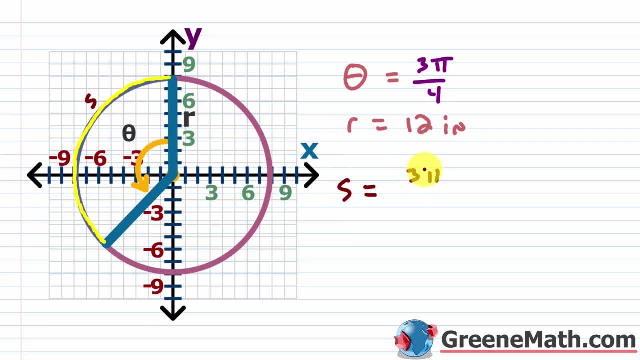 going to be equal to again. just multiply these guys together, So 3 pi over 4 times 12 inches. okay, And again, what's going to cancel here? 12 cancels with 4 and gives me 3.. So you're going. 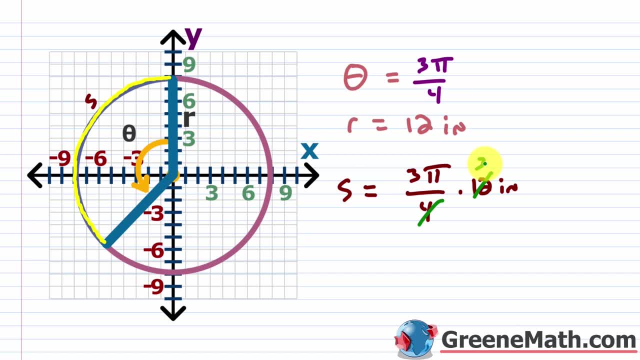 to have 3 times 3,, which is 9, times pi times inches. So you can say: well, I'm going to have this is 9,. okay, This is 9 pi inches. Again, you can write that out or leave it abbreviated. 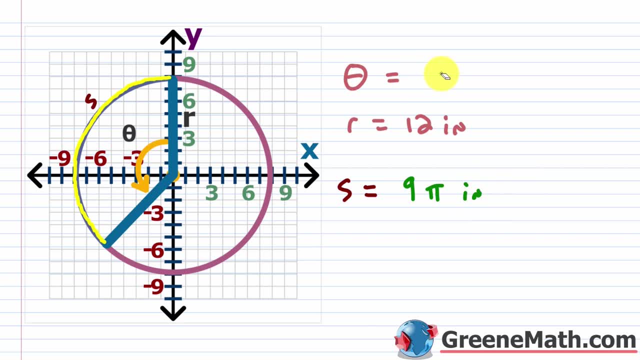 whatever you want to do, All right. So before we move on, I just want to talk a little bit about how you can do this with it being in degree mode. okay, It's a very simple formula, All you want to do. you probably remember this from geometry, but you just want to take 135 degrees and divide it. 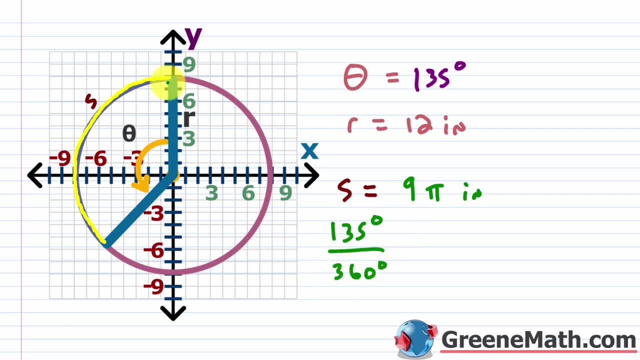 by 360 degrees. So, in other words, you're taking 135 degrees, which is the measure of this angle, okay, And dividing it by 360 degrees, which is the measure of one complete rotation, right, The angle that's formed by a complete circle. And then I would just multiply it by remember. 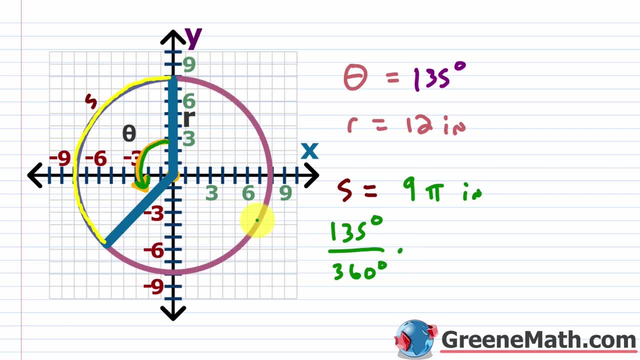 the circumference of the circle is the distance all the way around. okay, So the formula for that is going to be 2 times pi times r. okay, So if we do 135 degrees divided by 360 degrees, your units would cancel. 135 and 360 are each divisible by 45. If I divide this by 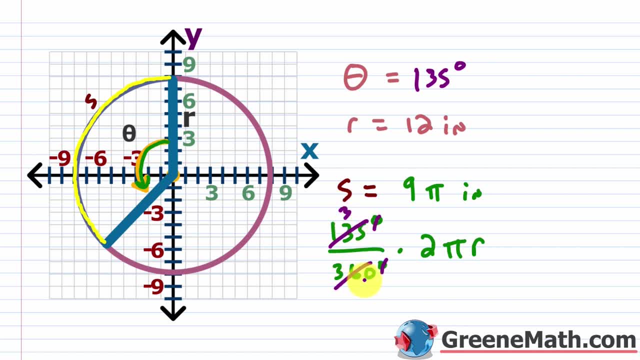 45, I get 3.. If I divide this by 45, I get 8, okay, So let's just write this as 3 eighths. Let's just write this as 3 eighths times this guy. So now I know that I can cancel this 8 with this 2. That. 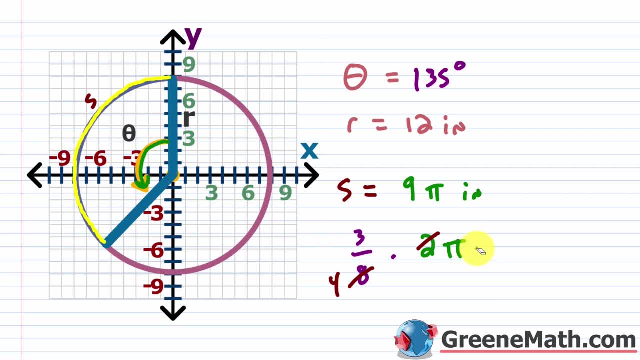 would give me a 4 down here. The r here, if I plug in for r, it's 12 inches, right? So this is times 12 inches. So what else can I do? I can cancel this 12 with this 4, and I'm going to get a 3.. 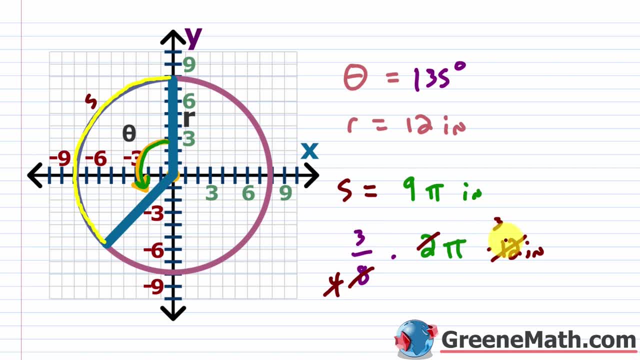 And if I multiply across, I'm going to get 3 times 3.. 3 times 3,, which is 9, okay, Times pi times inches. So I would still get an s that's equal to 9 pi inches. So it's the same thing and we can write it out and say that it's the same thing. 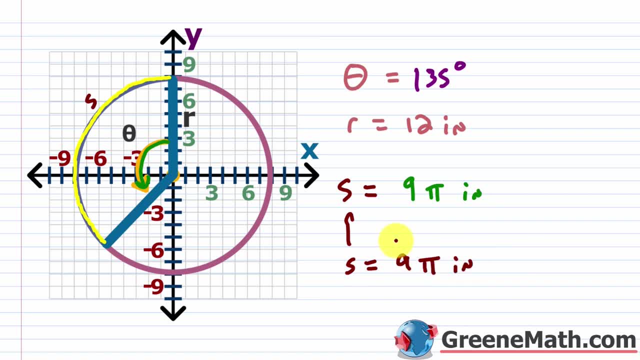 as this. So s is equal to 9 pi inches, right? So those guys are the same result. So either way you want to do this, it's going to give you again the same result. It's just a matter of which way. 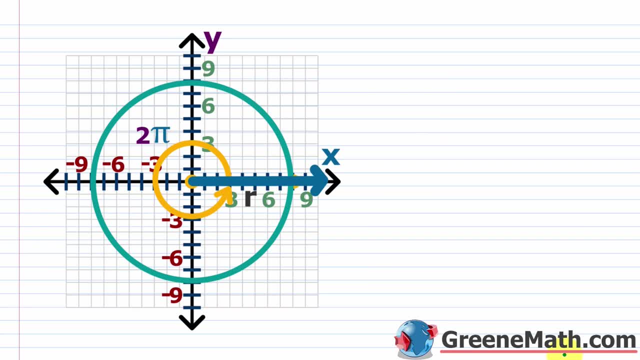 you prefer. All right, What we want to do now is talk about how to find the area of a sector of a circle. So we've already seen that a complete circle or one full rotation forms an angle with a measure that's 360 degrees, or in terms of 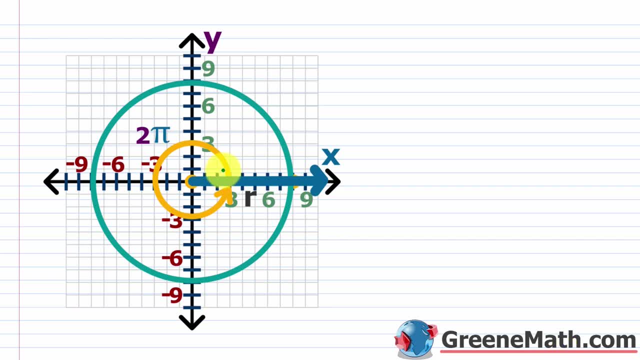 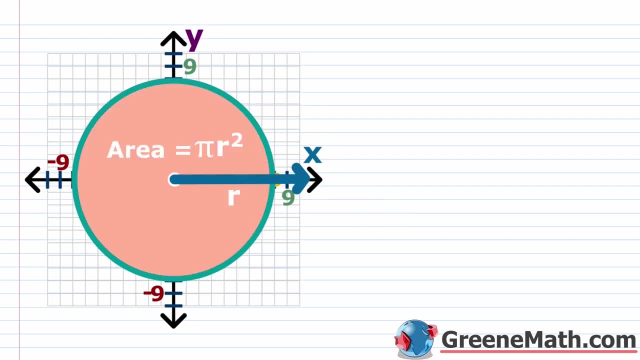 radians. it's going to be 2 pi radians. So you can see this guy: one complete rotation or one complete circle. it's 2 pi radians. okay, Now, if we think about the formula for the area of a circle- most of us know this from geometry- the area of a complete circle here is pi times. 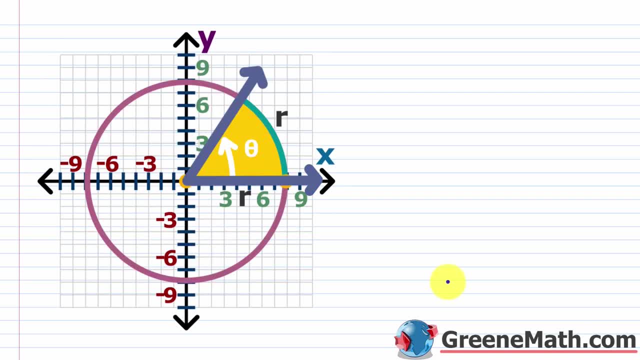 the radius squared. So now what if we wanted the area for a piece of the circle and we wanted the area for the circle? okay, So not the whole thing. So a sector of a circle is the portion of the interior of a circle intercepted by a central angle. So visually you can see on the screen. 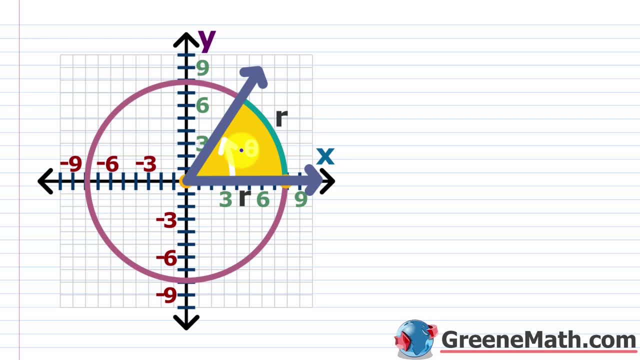 this looks like a piece of pi, okay. So how do we find, how do we find the area for this guy right here? Well, let's think about the formula and I'm just going to put a for area. Let's think about: 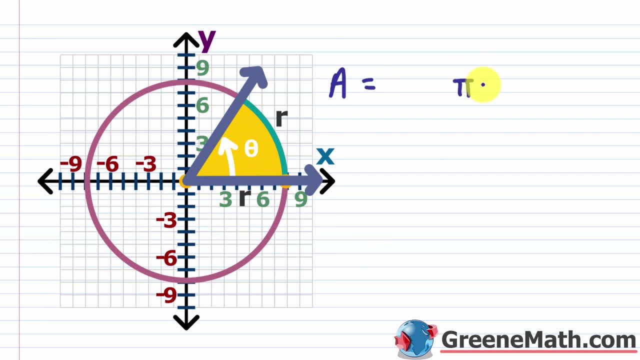 the formula for a whole circle. Again, it's pi times r squared, okay. So now that's for a 360 degree angle, we're getting radians 2 pi, Okay. so what I do here is: I think about the fractional amount of this guy, So I can take theta, okay, which is the measure. 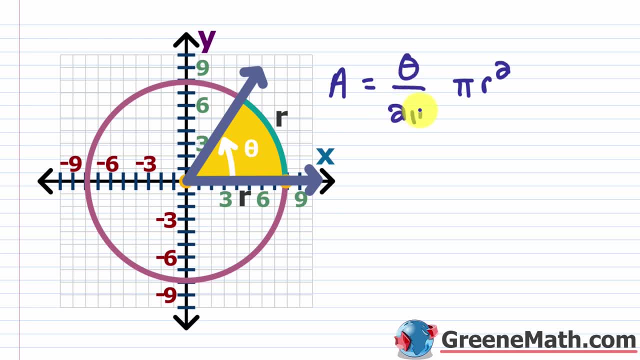 of this angle in radians and divide it by 2 pi, which is the measure of, again, a complete circle or one full rotation in terms of radians. So if I multiply this fractional amount here by this area of a circle formula, I'm going to be good to go okay. 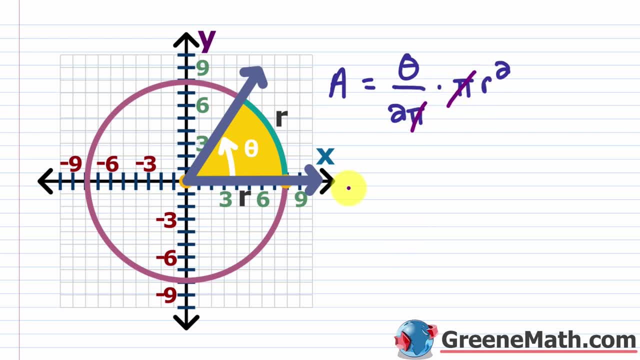 Now notice that you can cancel this with this and I can say that the area is going to be equal to what. Let's go ahead and say: this is one half times. we'll do theta times r squared, And there's different ways to write this, but most textbooks will write it in this way, So that's how I'm. 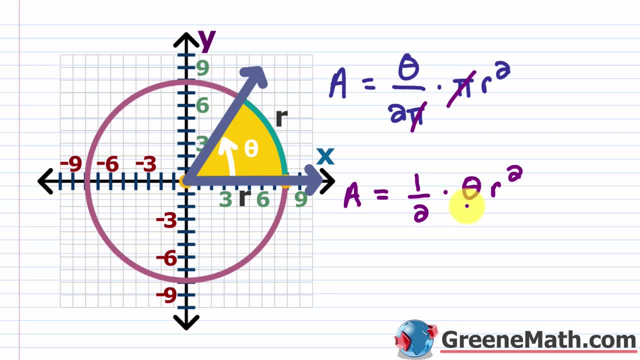 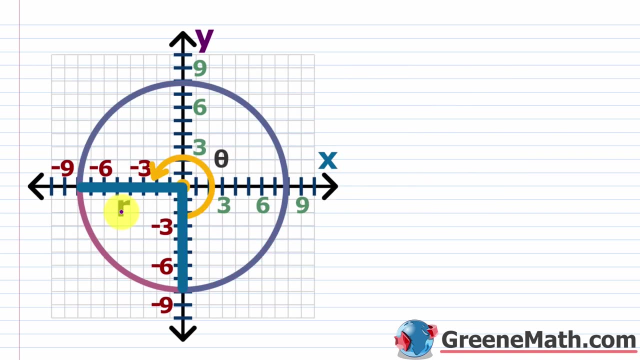 going to present it Now. what's important here is that theta be a central angle, okay, And that the theta also be given in terms of radians. If it's not, again you've got to convert from degrees to radians to use this formula. All right, let's take a look at an example. So we have our angle. 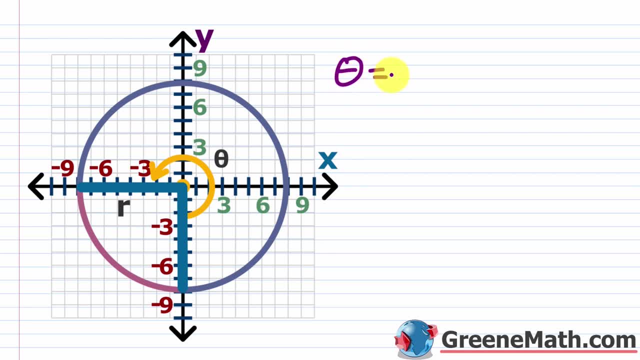 theta. we have our radius r. Theta is going to be given to us as 3 pi over 2.. The radius r is going to be given to us as 9 meters. You can write out meters or you can just put m for meters, That's. 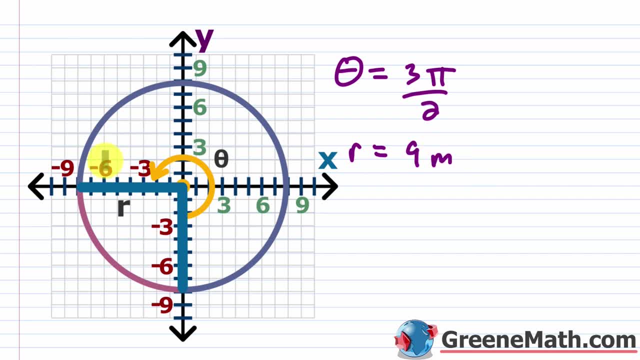 the abbreviation. And again, what are we trying to find? We want to find the area of inside of here. okay, And I'm not going to highlight this perfectly, but you get the idea. okay, So we're trying to find that area and let me just erase that. 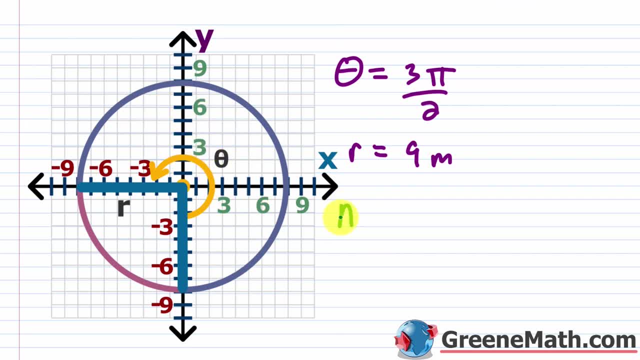 So how do we do this? Again, we're just going to use the formula. So again the formula here. you can write a for area. We'll say this is 1 half times r, squared times your theta, okay So? 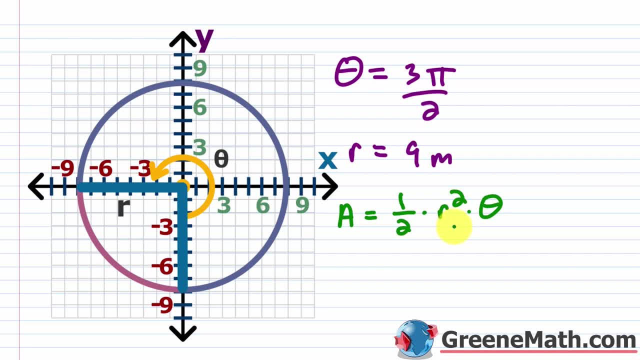 I'm just going to plug in What is r. in this case It's 9 meters, okay, So your area would be equal to 1 half times. I'm going to plug in 9m. m is for meters, and both of those are going. 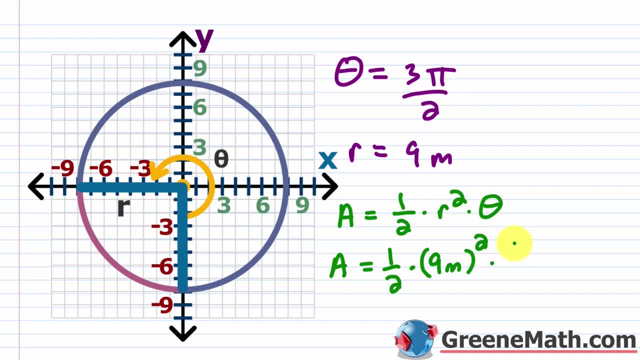 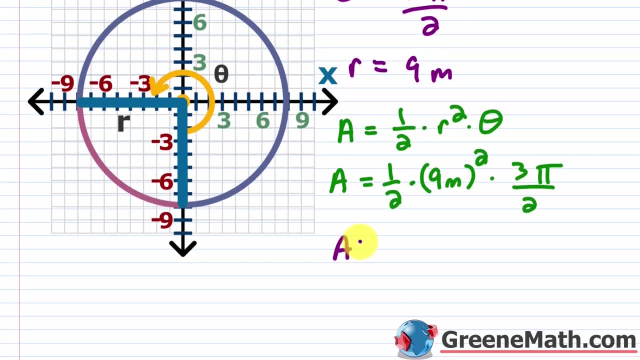 to get squared- Remember you've got to square your units as well- And then times your theta pi over 2.. Let me scroll down a little bit and get some room going. So my area here is 1 half times the 9 gets squared, it's 81, the meters get squared, So you could write this as square. 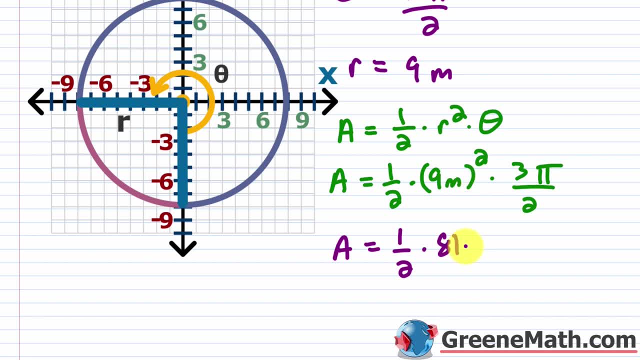 meters or meters squared, or you just put m squared for short, So m squared, and then times your 3 pi over 2.. Okay, so can we cancel anything? No, it doesn't look like we can, So we're going. 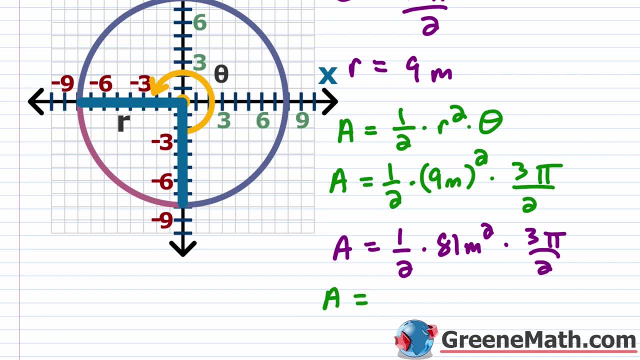 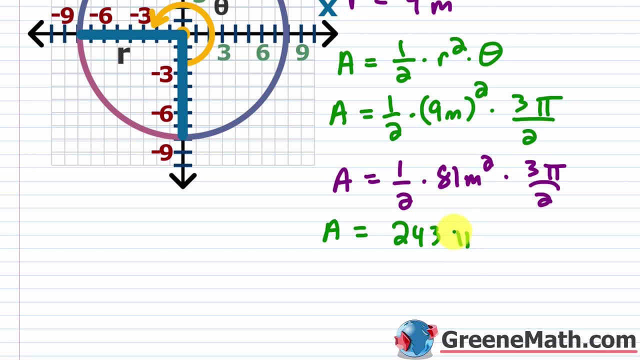 to say that the area, the area is going to be equal to. we're going to say that 81 times 3 is 243,. okay, then times your pi and then this will be over. 2 times 2 is 4, and this will be in. 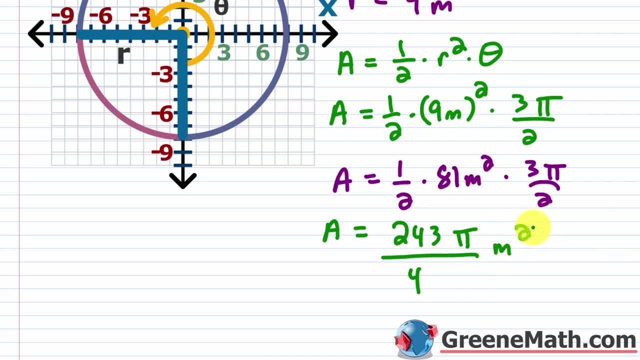 terms of square meters, where you can just write m squared. Again, m is the abbreviation for meters and we know it's being squared. okay, So you could write meters out and square it like that. you can put square meters or meters squared if you want to write it out. Any of those would work. 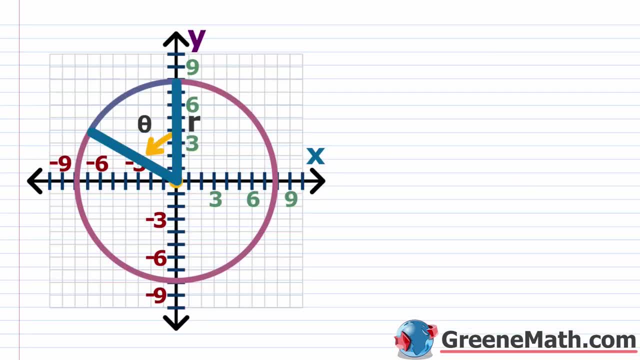 but make sure that you square the units and you show that in some way. All right, let's take a look at one more. So suppose now that theta is given to us as 60 degrees and the radius r is going to be given to us as 13 yards. So I'm going to put yd to. 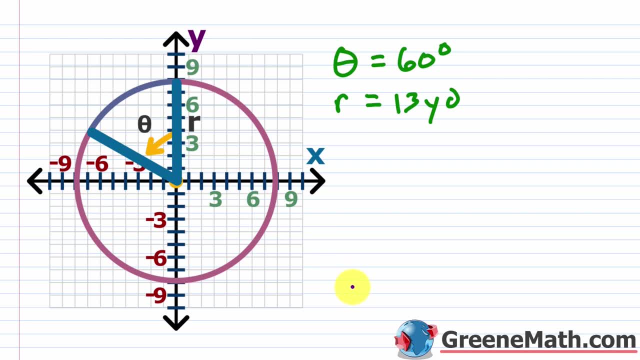 abbreviate yards. So let's go ahead and say that the area again is equal to one half times your theta times your radius squared. Now again, theta has to be given in terms of radians. okay, So we need to convert this guy into a radian measure. So I'm going to take 60 degrees. 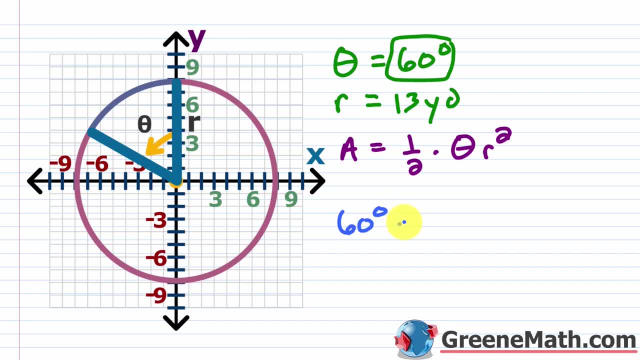 and multiply it by. remember pi radians equals 180 degrees. So I'm going to put pi up top, I'm going to put 180 degrees at the bottom and I'm just going to cancel, okay, So this would. 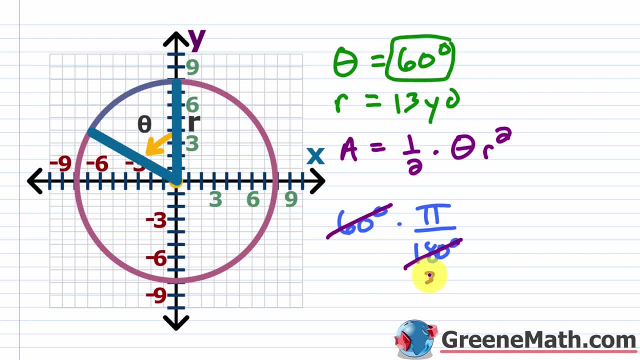 cancel with this and leave me exactly three, okay, So this would be pi over three. this would be pi over three, okay, So let's erase this and let's think about this now. So we're going to. 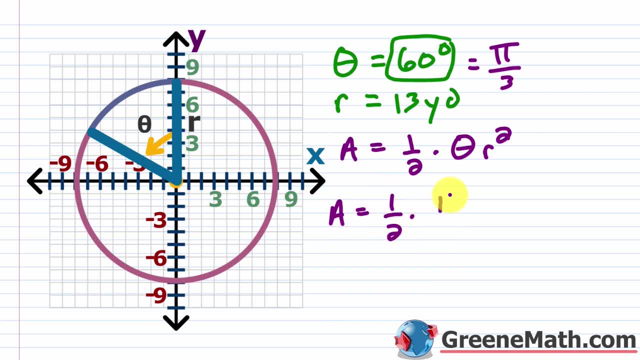 have. the area is equal to one half times. you've got your pi over three times the radius, which are the yards being squared, So don't forget about those units. it's very important. So we're going to say that the area is equal to. can anything cancel? No, So I'm just going to go. 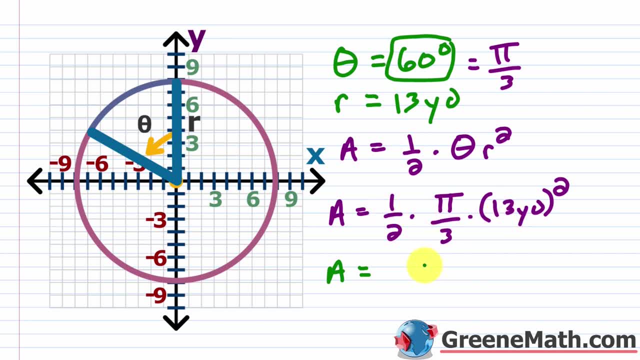 ahead and say that 13 squared is 169. So this would be 169 times pi. okay, I'll deal with the yards in a moment over your six. and then yards squared Again. you could write square yards. you could write yards squared however you want to do this. I'm just going to put yd for the. abbreviation of yards, and then I'm going to put a squared as well. All right, that's everything for the other part of the equation. So what do you want to do with this When you're adding yards? this is what I'm going to do. So instead of adding plus and minus, I'm going to add a squared and penis. 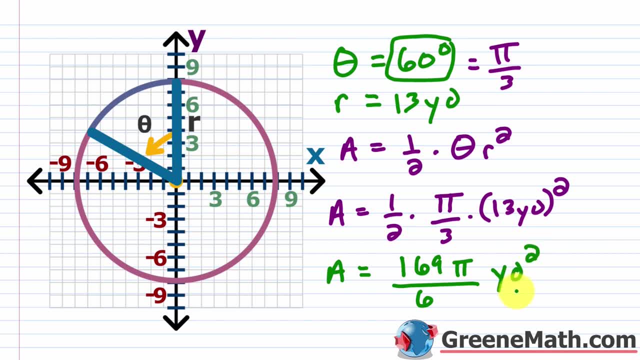 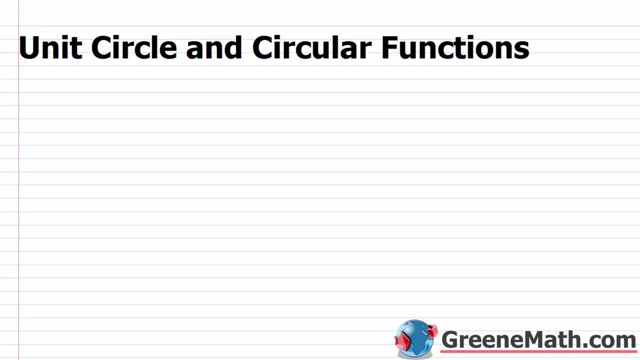 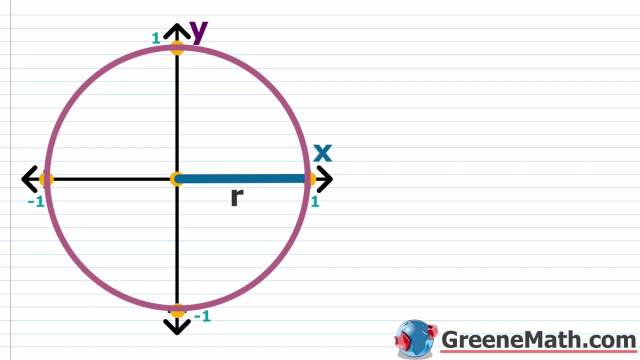 and then I'm going to put a squared like this. So the area here would be 169 pi over 6 square yards, or again yards squared. In this lesson we want to talk about the unit circle and circular functions. All right back in our algebra course we learned how to graph a circle. 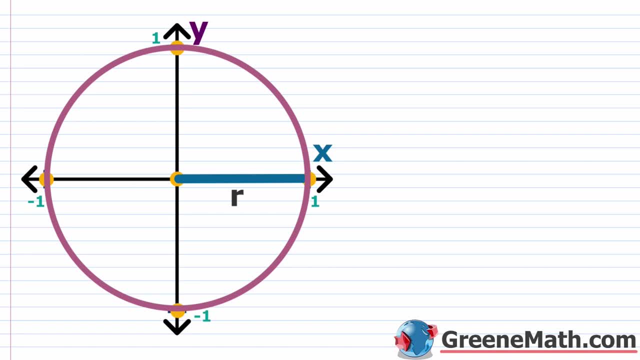 and we also learned how to work with the equation of a circle. So we have here a unit circle and the center here is at the origin and the radius is going to be 1.. So the equation for this circle is going to be: x squared plus y squared is equal to 1.. So again, this has a center at the origin. 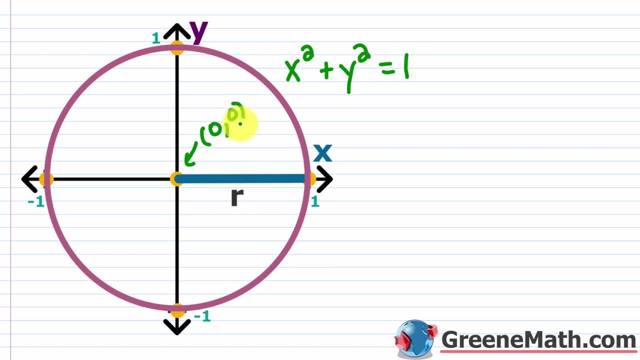 so there's my center, it's at the origin, it's going to be the point 0 comma 0 and my radius is going to be 1.. So that tells me that the distance from the center to any point on that circle is going to be one unit. Okay, so from the center here to this point here, if I move one unit to the right, 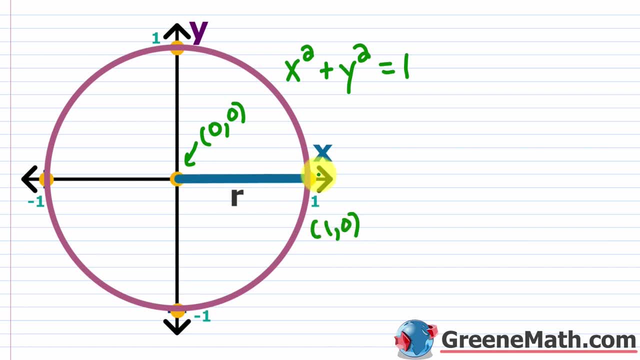 this is the point 1, comma 0.. Okay, so I've moved just one unit to the right. If I move from the center one unit up, this is the point 0, comma 1.. If I move from the center one unit down, this is the point 0. 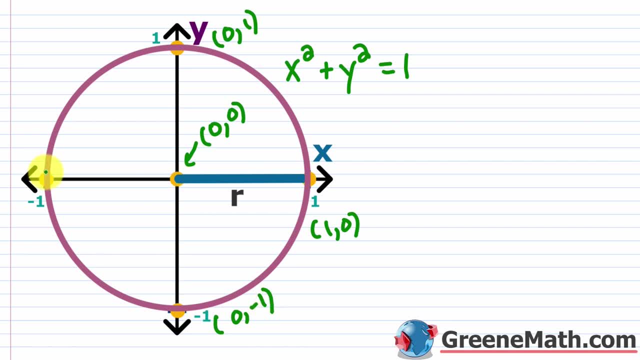 comma negative 1.. And lastly, if I move from the center one unit to the left, this is going to be the point negative 1 comma 0.. Okay, but the main thing to understand is that the distance from the center to any point on that circle is one unit. Now, using the unit circle to work with our 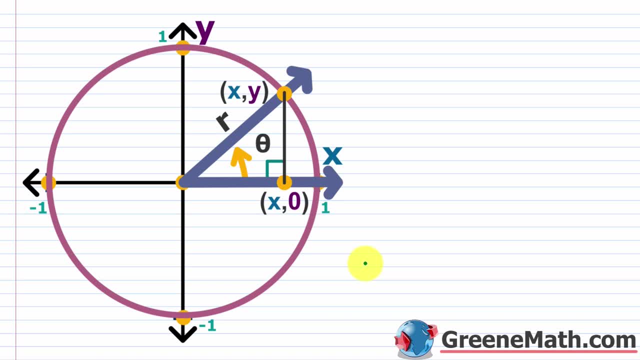 trigonometric functions will lead to some interesting results that allow us to quickly solve problems as we move forward in trigonometry and also into calculus. So let's just get started here. on our unit circle, We have an angle that's in standard position, So basically, this is the 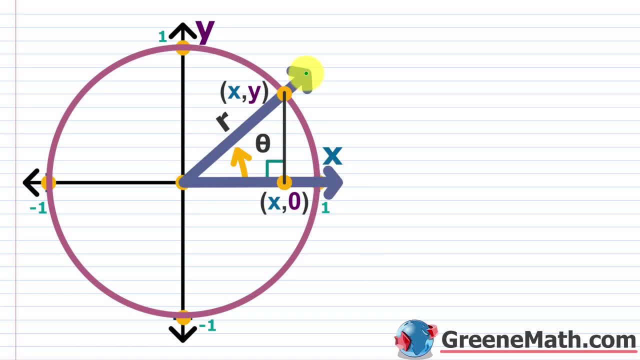 initial side and this is your terminal side. So your terminal side of this angle, theta okay- is going to lie in quadrant 1.. And notice, we have a little point here and this point is going to be labeled as x, comma y, just generically. you could use a, comma b or whatever you want, And that point. 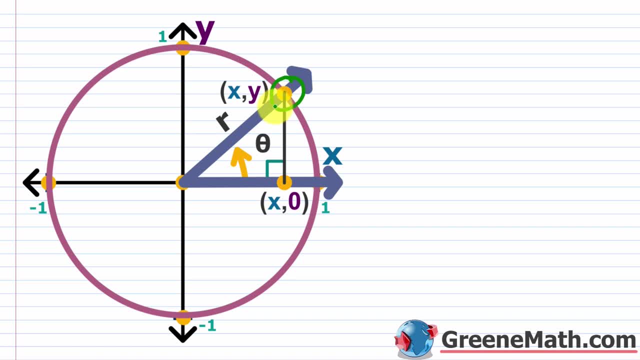 there is going to lie both on the unit circle and on the terminal side of our angle. So if we wanted to find something like sine of theta, so sine of theta, what would this be? Well, we know, when we started this course, we had a. 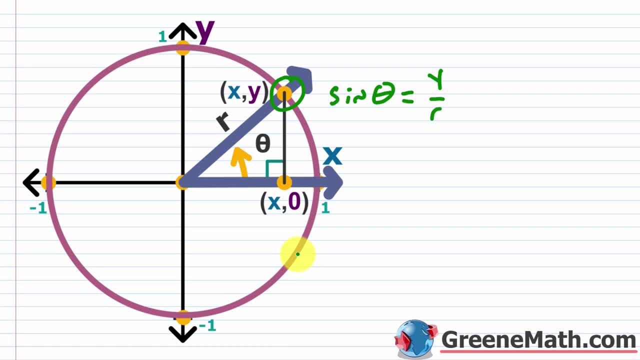 definition that was y over r. But you could also use opposite over hypotenuse, it doesn't matter, you're gonna get the same thing here. But basically we know that this guy right, if we look at this guy from here to here, this has a length of y, right, because this coordinate is y, this coordinate. 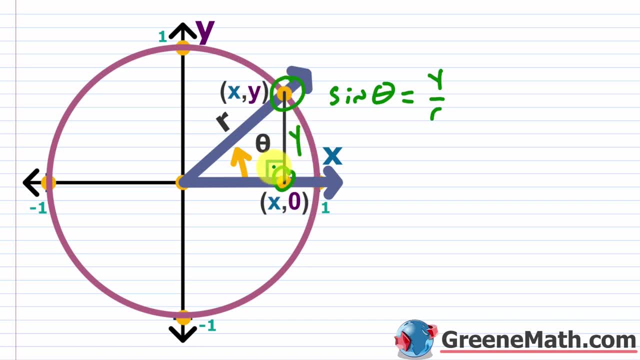 is zero, right? So this vertical distance here, this vertical distance here, is y, Right, y minus zero. that's all you're doing. So if I think about this r, the radius which is my hypotenuse here, okay, is going to be one, right, because we're on the unit circle. the radius is: 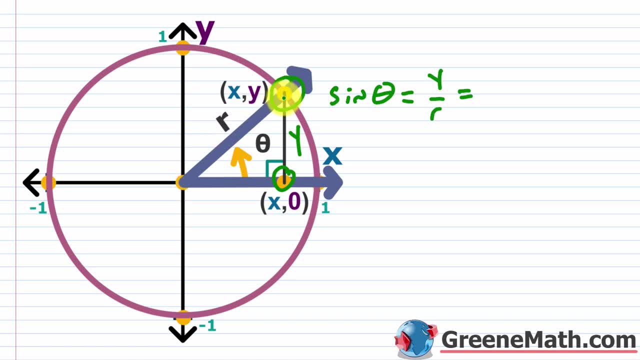 one. So again, the distance from the center to any point on that circle is one. So, sine of theta is going to be y over r, which is y over one, which is just y, okay. So sine of this angle, theta is: 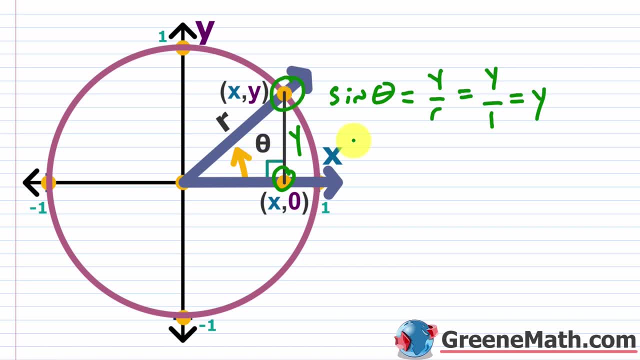 just going to be the y coordinate of this point right here, okay. And then the same thing is going to happen when I work with cosine of theta. Remember, this is x over r, or again you could say adjacent over hypotenuse. okay, And in this: 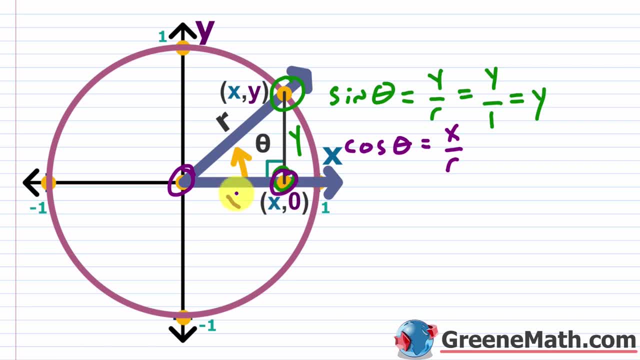 case, the length here, from right here to right here, is going to be x. okay, So it's just x over r, which is x over one, which is x. So the cosine of theta is just going to be the x coordinate for. 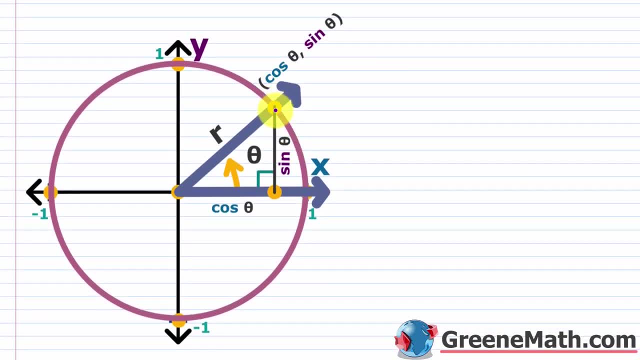 this point right here. So what we can do is really label this point right here as the cosine of theta and then the sine of theta. So again, this is your x coordinate and this is your y coordinate. So let's quickly talk about the concept of circular functions. Basically, all we're going to be doing. 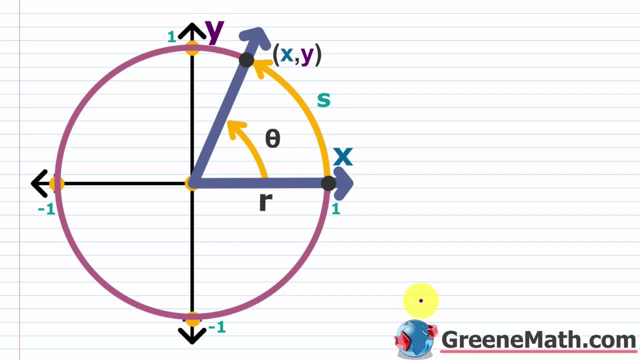 here is swapping out theta for s, okay. So how does this work? Well, when we're working with a unit circle, remember that the radius is one, The formula for our angle, theta in radians. remember it comes as theta is equal to s, which is the length of the arc. okay, divided by r, which is: 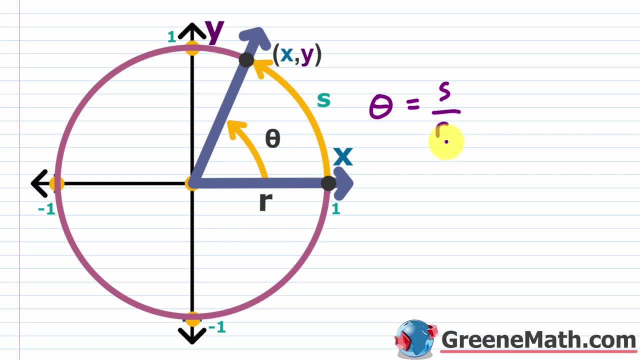 your radius. Well, in this case the r is one. okay, The r is one, So theta will be equal to s. So when we're on the unit circle, our trigonometric functions of our angle, theta measured in radians, found again by choosing some point, x, comma, y on the unit circle, can now be rewritten as functions. 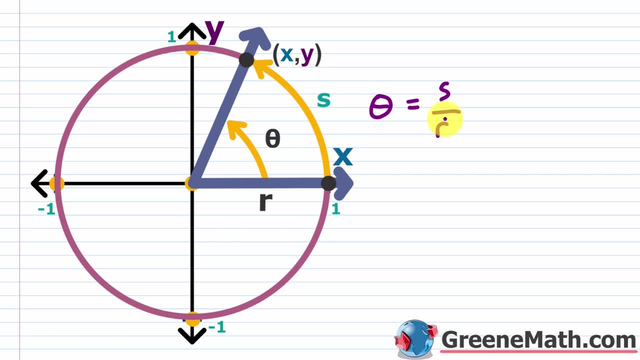 of the arc length s, some real number. okay, So when we show it in this way, the functions are known as circular functions, So you'll probably see this in your book. They're going to use this letter s instead of theta, right? So they'll start saying: sine of s is equal to y, and then 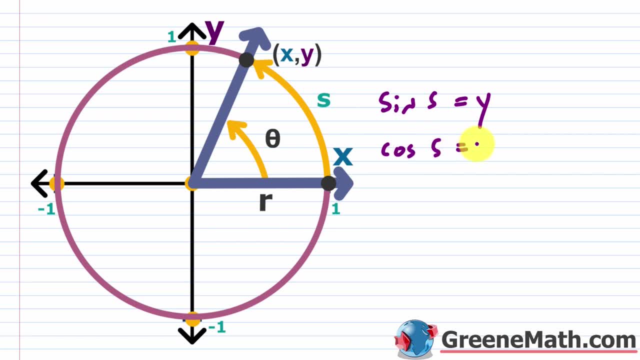 cosine. cosine of s is equal to x, and then you can get the rest of them using these. So you could say: tangent of s is going to be y over x, and then you can get the rest using the reciprocal identities, right? So the cosecant of s is one over y, the secant of s is one over x and the 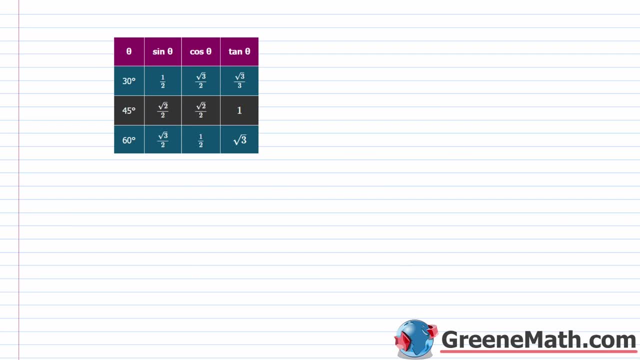 cotangent of s is x over y. All right, so let's talk about how we can set up our unit circle now. So we're going to rely on these trigonometric function values of special angles, right, We've talked about this before. So we know, and I'm just going to go through a few of these. So the sine of 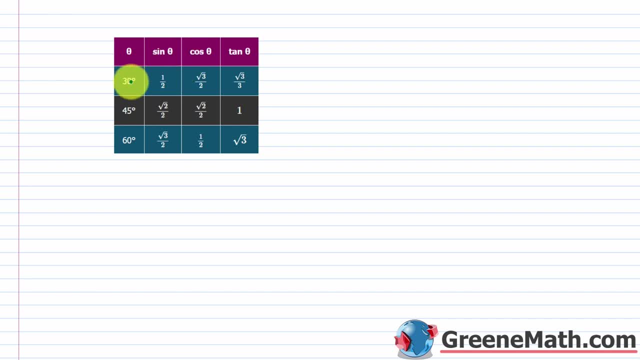 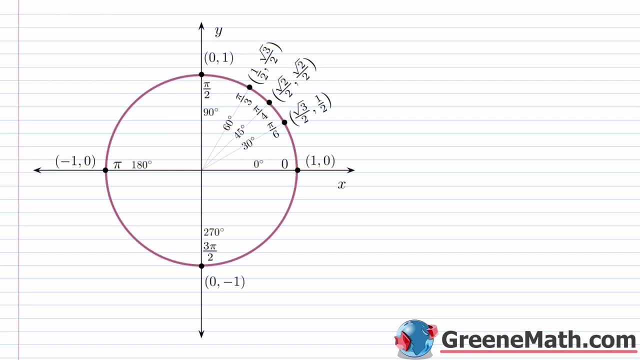 30 degrees is a half and we know the cosine of 30 degrees is square root of 3 over 2.. So let's just take that real quick. Let's go down to a sample unit circle. It's not all filled out, just part. 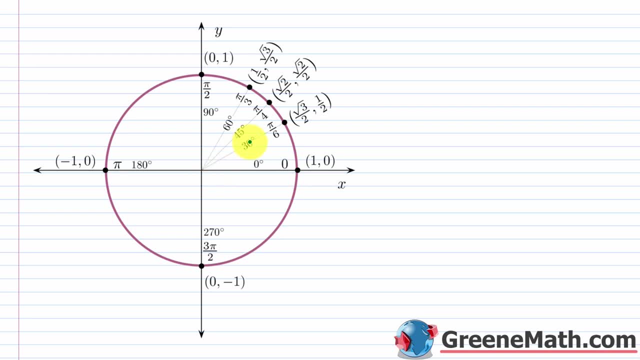 of it so I can show you where things are coming from. And if we look at a 30-degree angle, which is, in terms of radians, is pi over 6, we see that the x squared is equal to y over x and the cosine. 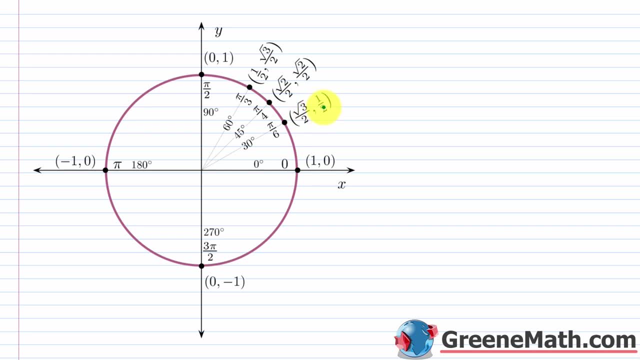 is a square root of 3 over 2, and the y coordinate is one half. Remember, because we're on the unit circle, we have this property, This x coordinate here is the cosine of this angle. You could say it's 30 degrees, or you could say it's pi over 6 radians. whatever you want to use, it doesn't. 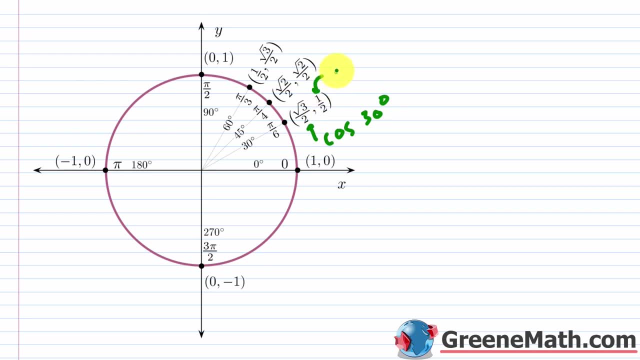 matter. And in this case the sine here is going to be your y coordinate. So the sine of 30 degrees is one half, that's your y coordinate. Again, the cosine of 30 degrees is your x coordinate. it's square root of 3 over 2.. So using the same logic, you can see that if I'm working with a 45, 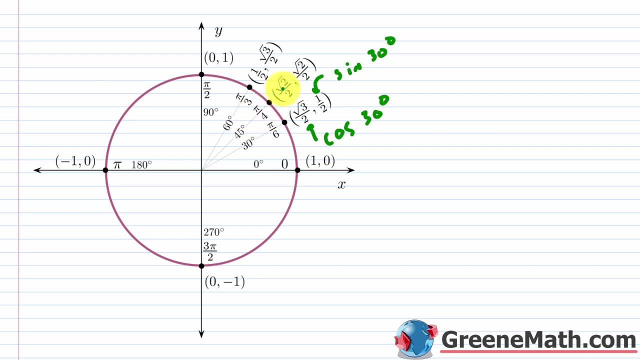 degree angle or pi over 4 radians, this would be my cosine and this would be my sine. If I'm working with a 60 degree angle or pi over 3 radians, this guy right here, this would be my cosine, the one half and this would be my sine, the square root of 3 over 2.. So the point that's: 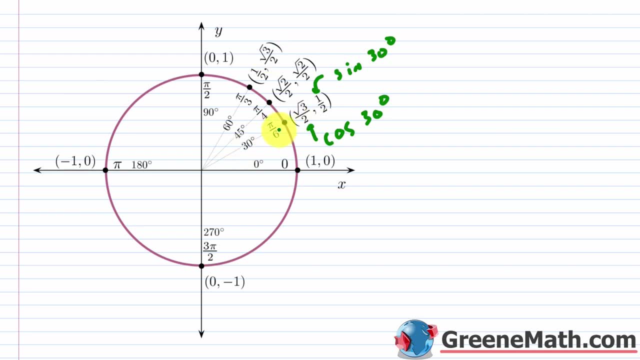 associated with that angle. the x coordinate is the cosine, the y coordinate is the sine. So very simple. So once we have this guy set up, there's a lot of different tricks or techniques to remember these three different values. here Some people use the hand trick. there's all kinds of stuff out. 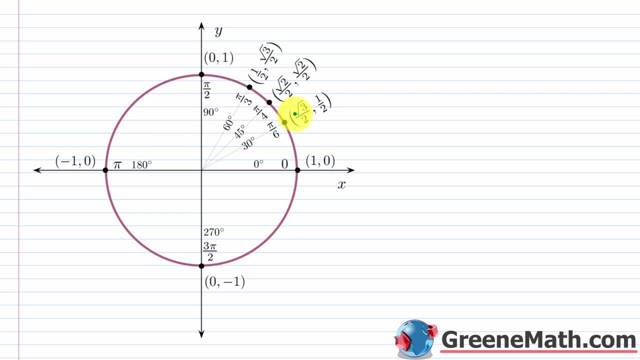 there I'm going to show you what I learned a long time ago. There's a lot of videos that do it this way as well. What you'd want to do is set up in each case a denominator of 2.. So a denominator. 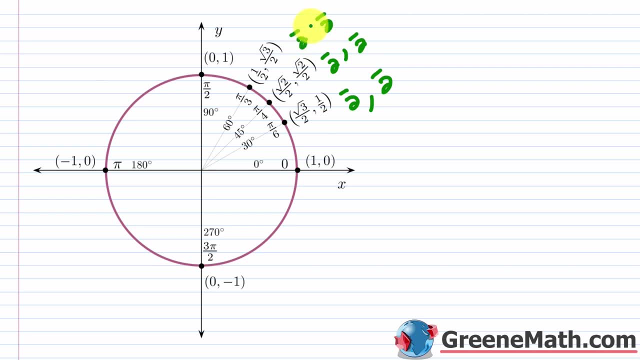 of 2, a denominator of 2.. Okay, so that's going to be everywhere. You'll notice you have 2, 2,, 2,, 2,, 2, 2.. That's very easy, Remember, okay. Then the next thing you want to do: you'll notice that if you ignore the square, 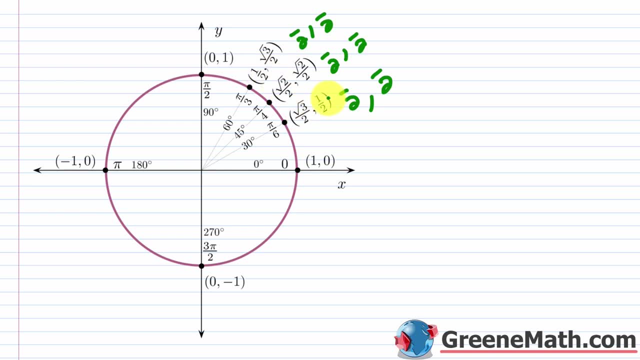 root symbol. you start here with 1 and you're counting down. and you start here with 1 and you're counting up. So I'm going to make all the numerators like this, So 1,, 2,, 3, and then I'm 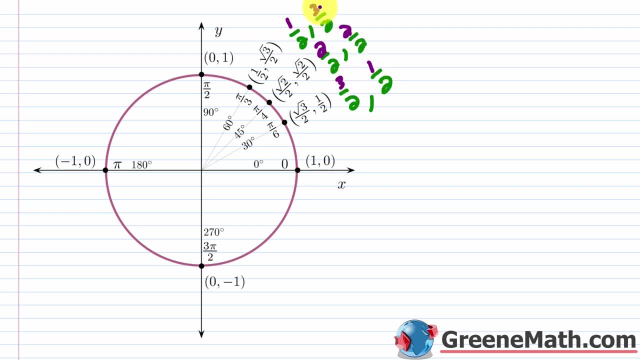 going to go 1,, 2, 3.. Okay, if you get lost about where you want to put the 1 and start and go down, all you need to do is think about: okay. well, if I'm going from right here to right here, 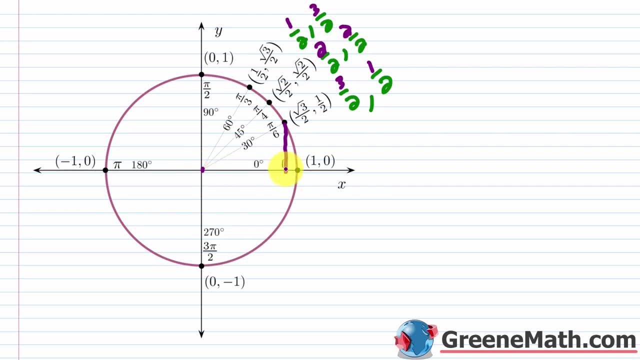 triangle, this x distance is greater than this y distance. Okay, so that tells me that I would want the 3 here. I know it's square root of 3, but just forget about the square root symbol for now. I know this would be greater than this, So I would start with a 3 here, or you could say I'd start. 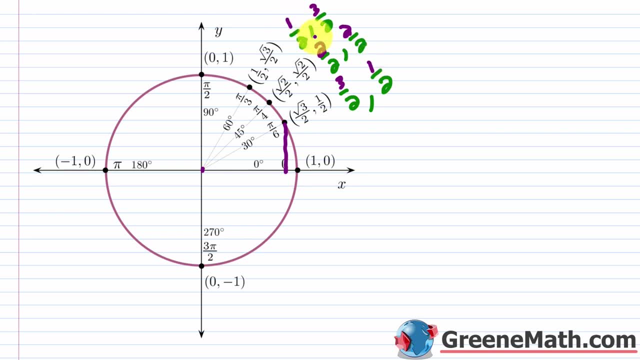 with a 1 here. However, you want to remember that you're going to have a 1,, a 2, and a 3, and then a 1,, a 2, and a 3.. Okay, so that's a little technique you can use. There are many others. 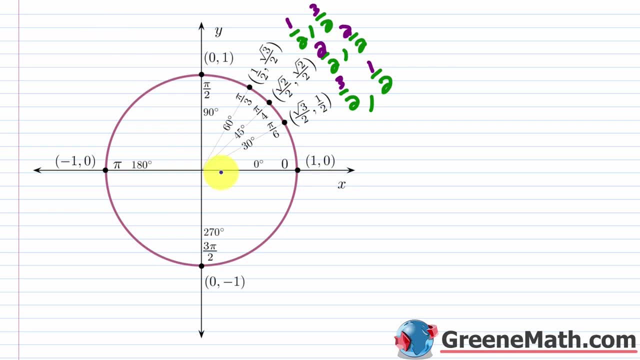 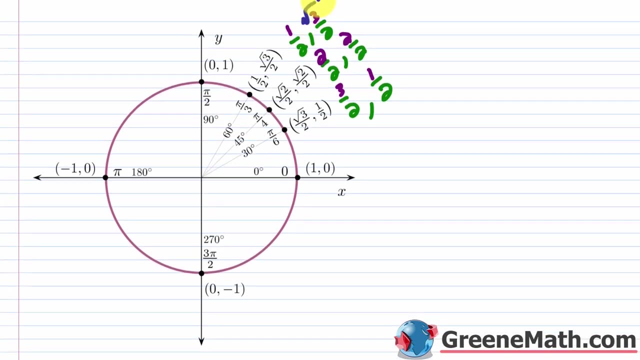 that you can go with. Now, once you're finished with that, you want to square root all of the numerators? Okay, and if you have the square root of 1, remember that's 1. So you can skip those. So I'm going to have square root of this, square root of this, square root of this, and 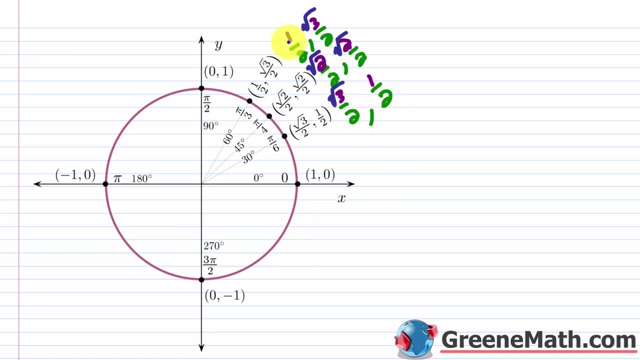 square root of this. Okay, remember the 1 here. the 1 here, square root of 1 is just 1, so you can just ignore it. Okay, so now we have all of these guys, You can wrap it in parentheses to make it. 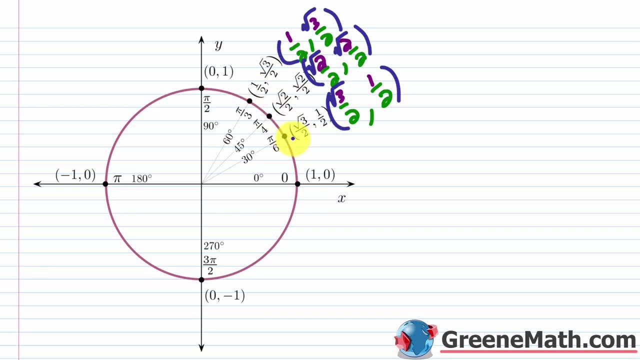 official, if you want, but that's how I get these points there. So, now that I have all of these points, what I want to do is reflect across the y-axis to get these points over here. So let me show you this And, basically, if I'm reflecting across the y-axis, think about this for a moment. 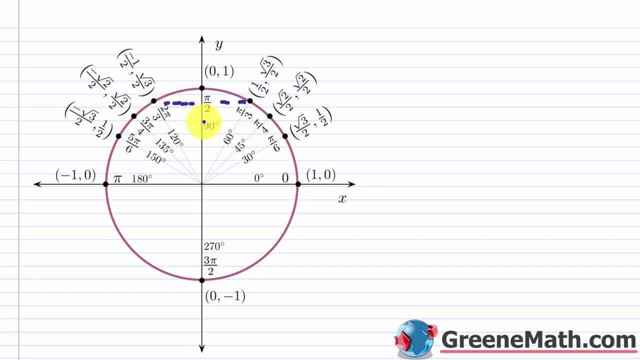 If I go across the y-axis like this, the y-coordinate is the same. Okay, so you'll notice: here you have square root of 3 over 2, and here you have square root of 3 over 2,. so that's the. 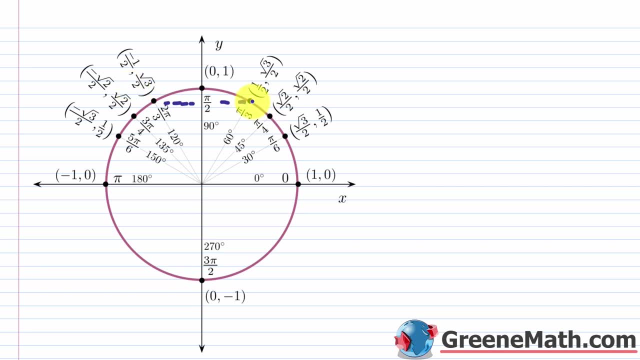 same. The x-coordinate is now its opposite right, because I'm on the opposite side of the y-axis. Over here, x values are negative. Over here, x values are positive. Okay, so this is negative. 1 half now instead of 1 half. This is negative square root of 2 over 2 instead of square root. 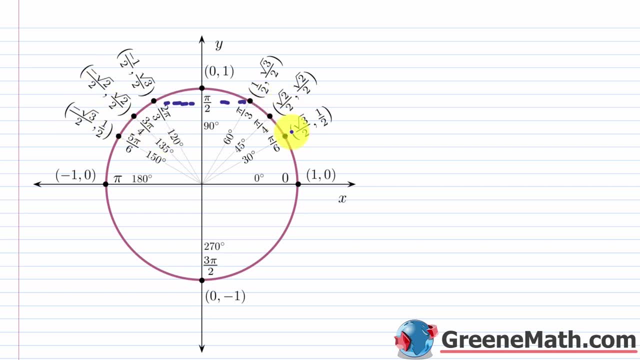 of 2 over 2.. This is negative square root of 3 over 2 instead of square root of 2 over 2.. This is negative square root of 3 over 2 instead of square root of 3 over 2.. Okay, so it's very. 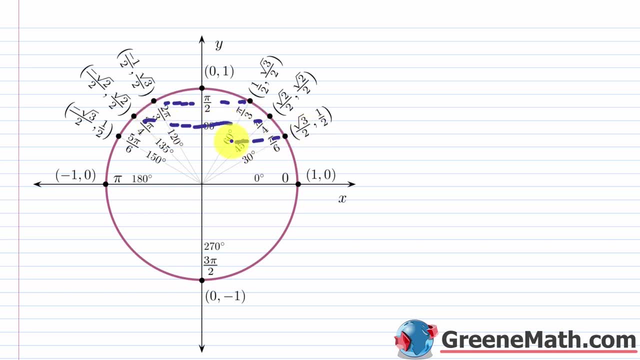 easy to just reflect these guys across. Okay, and I know these lines I'm drawing are not perfectly straight, but just pretend they are. So once you've done that now, you can reflect these guys across the x-axis and you'll have all your points. Okay. so now, if you think about a point, 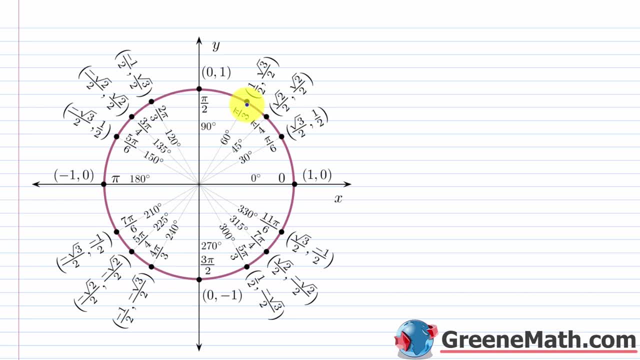 that's up here. if I reflect it across the x-axis, the x value will be the same but the y value will be its opposite. So if I reflect this guy right here, I'm going to have a point that's here down there and I know that line's not perfectly straight, but you have 1 half. 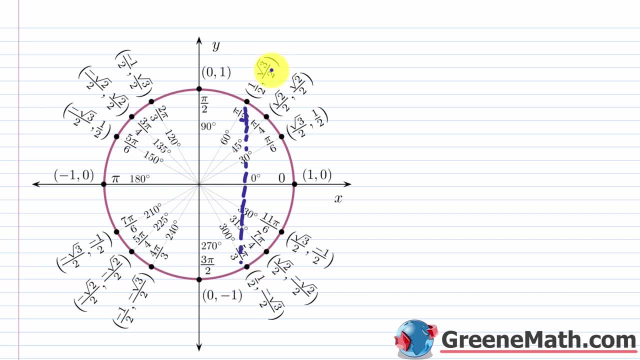 and you have 1- half, So the x value is the same. Then you have square root of 3 over 2, and then the negative square root of 3 over 2.. So that's all we're doing here: to get these values Again. if you can just remember these values in the first quadrant, okay. 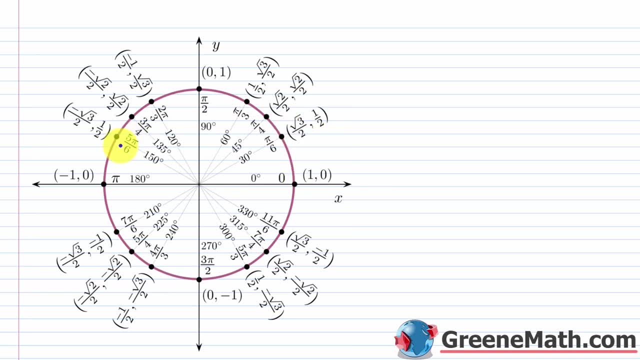 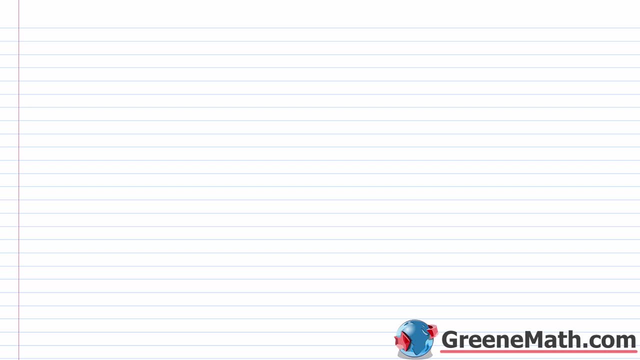 you're going to be good to go. You can use the reflection, okay, across the y-axis and then across the x-axis to get all the remaining points, Okay. so let's go ahead and do this. Let's go ahead and take a look at just a few examples. So I want to look at the sine. 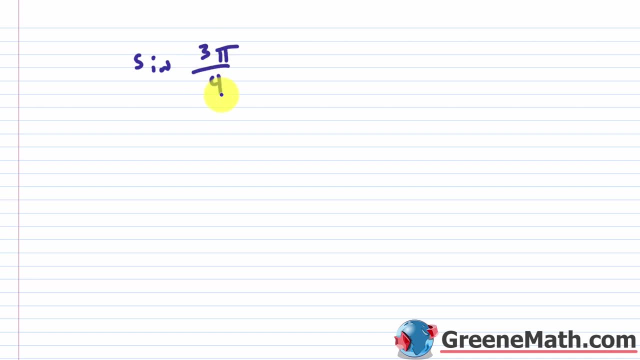 of 3 pi over 4, and then I want to look at the cosine of 3 pi over 4, and then, lastly, I want to look at the tangent of 3 pi over 4.. Okay, so we know that we could solve this. 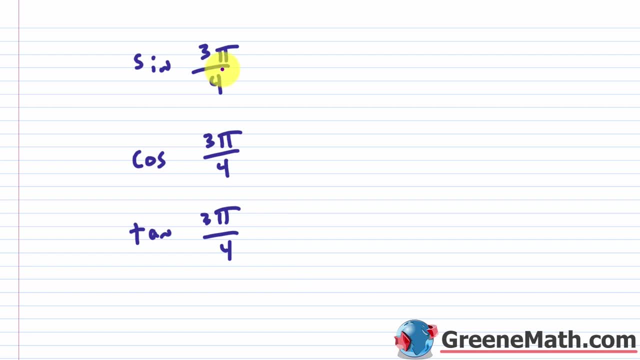 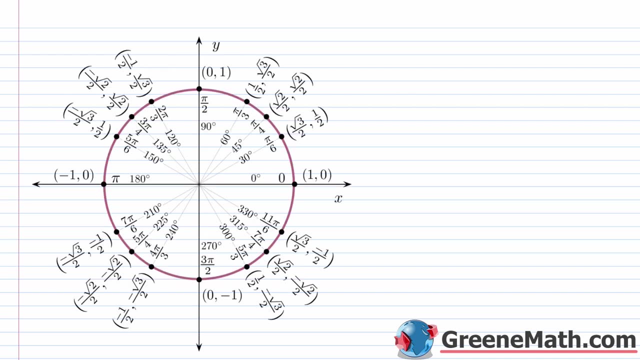 using methods without the unit circle- right, We already know how to do this, But using the unit circle it's going to be a little bit quicker. So I'm going to find 3 pi over 4. On my unit circle. So where is that going to be? 3 pi over 4 is going to correspond. 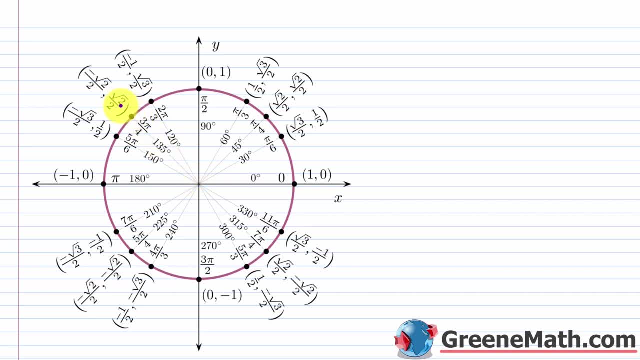 to a 135 degree angle. So it's this guy right here, And you can see that you have the negative of the square root of 2 over 2.. So that's your cosine. Let me write that out: Your cosine of 3 pi over 4 will be equal to the negative of the square root of 2 over 2.. And then you 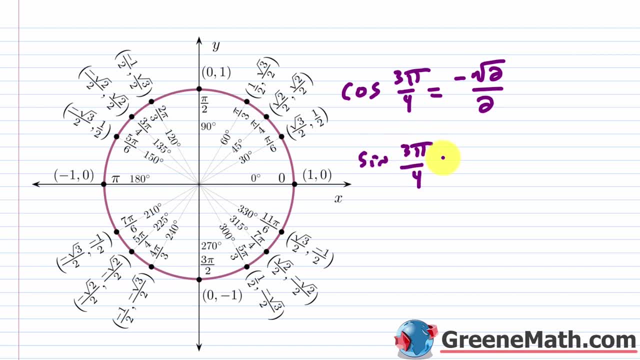 have your sine of 3 pi over 4 is equal to the square root of 2 over 4.. So that's going to be 2 pi over 4.. So this is the squared root of 2 over 2.. Okay, So let's copy this. 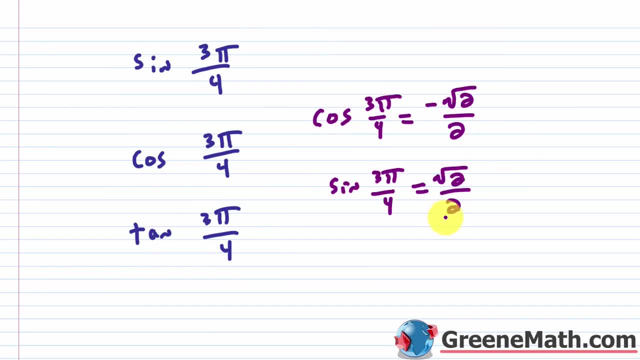 real quick. Come back down here. I'm just going to paste this in, So let me just rewrite this. So this would be the square root of 2 over 2.. And this guy would be: let me just erase this, I'm going to just drag this over. It's the negative square root of 2 over 2.. 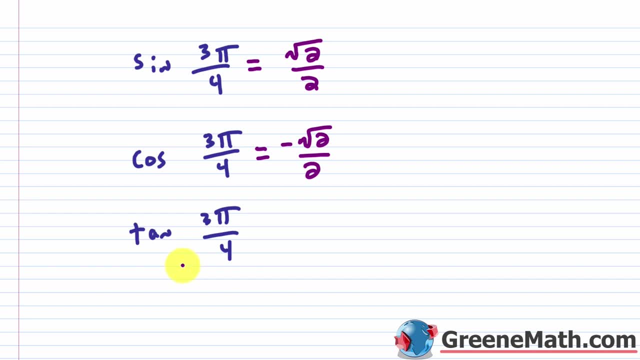 Okay. so how do I get my tangent here? Well, remember, the tangent is found by taking the sine and dividing it by the cosine. So I would take the square root of 2 over 2, and divide it by this guy. But if I'm dividing fractions, I want to multiply by the reciprocal, So I'm going. 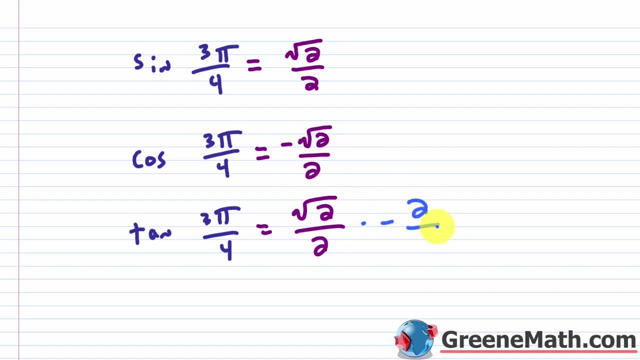 to flip this guy. I'm going to put the negative out in front. I'm going to flip this guy and put two over the square root of two And you're going to notice that this will cancel with this. This will cancel with this And you're left with negative one. Okay, So my tangent of three pi. 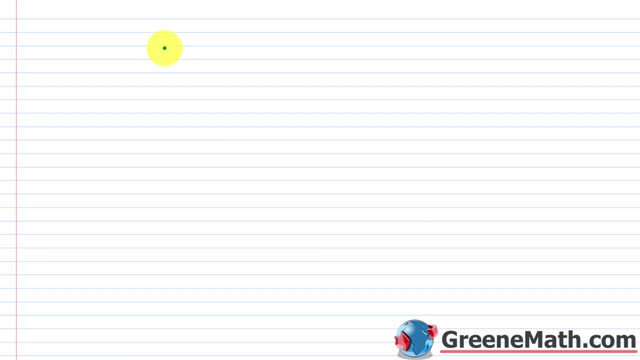 over four is negative one. All right, Let's take a look at another example. So suppose we had something like the sine of: let's say 13 pi over six, And let's also do the secant, the secant of 13 pi over six, And let's also do the cosecant, the cosecant of 13 pi over six. Okay, So if you 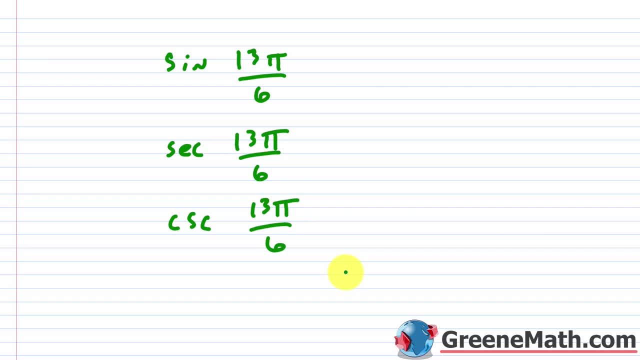 get an angle that measures that's larger than 360 degrees or two pi in terms of radians. again, what you want to do is find a coterminal angle that's between zero degrees and 360 degrees, or zero and two pi radians. So if I'm working with radians, what I'd want to do, let me just kind of divide this workspace up. 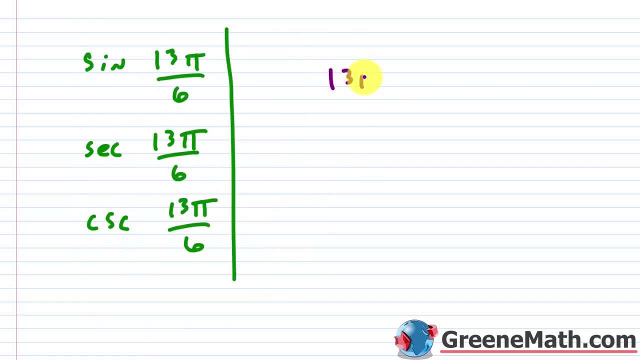 here And I'll just move this over for right now. What I want to do is say I have 13 pi over six radians. If I subtract two pi away, I would get a common denominator. So I'd multiply this by six over six. So this would end up being what It would end up being: 12,, 12 over six, right, 12 over six. 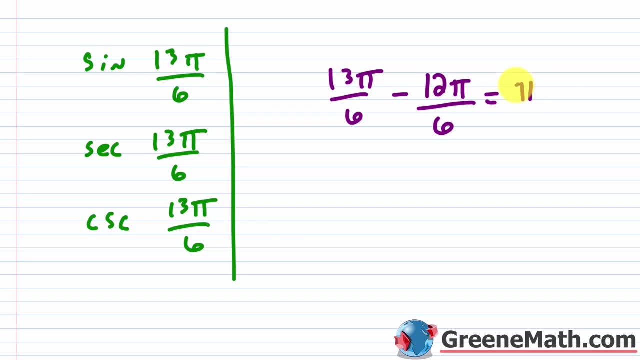 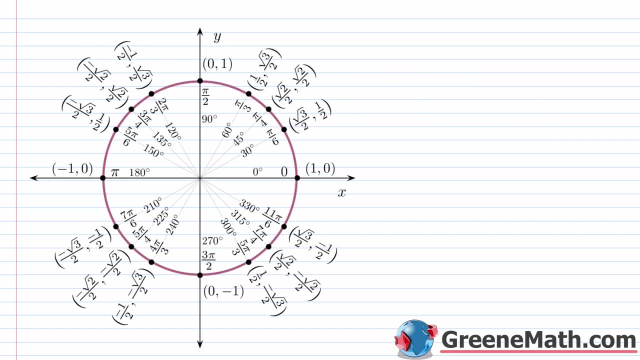 is the same thing as two, So what I'd have here is pi over six radians. Okay, So I would look at pi over six on my unit circle and that's going to be right here. Okay, So this is pi over six. 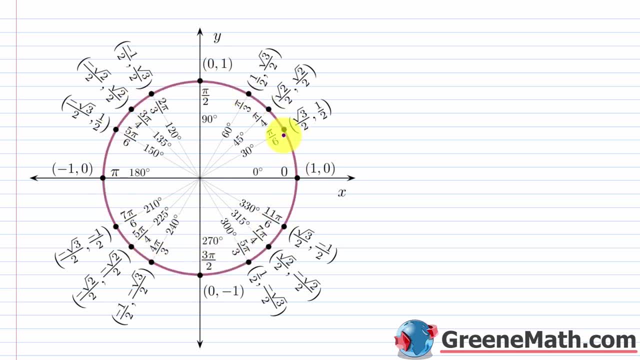 Again. if I went one more revolution around, I would end up with an angle that has a measure of 13 pi over six radians, or 390 degrees. Okay, So my cosine of pi over six is going to be the square root of three over two, And then my sine of pi over six is going to be: 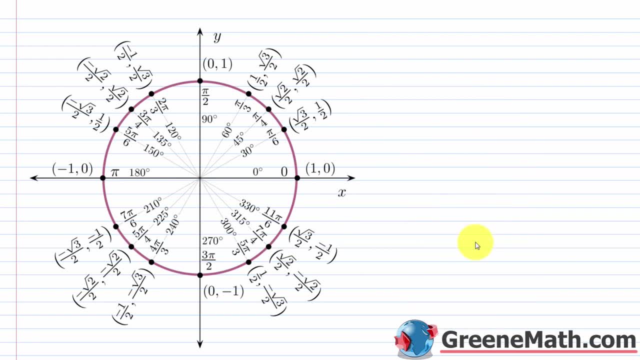 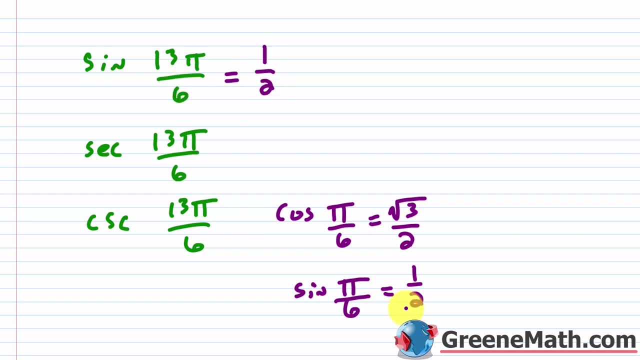 one half Okay. So let's go ahead and copy this, And so I'm going to write that the sine of 13 pi over six is going to be one half Okay, Because it's exactly equal to this here. Then for the: 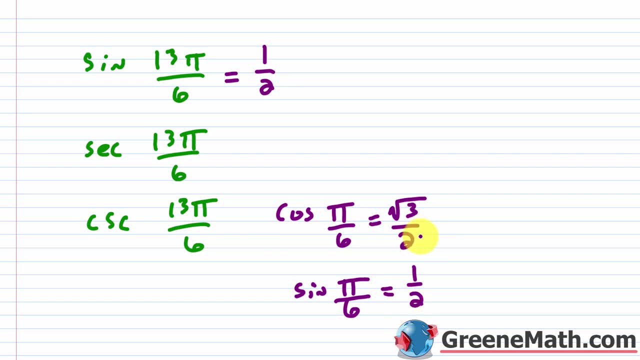 secant. it's the reciprocal of my cosine. Okay, So this would be equal to. I would flip this guy, I would have two over the square root of three over two, And then I'm going to write that the square root of three. Okay, And you just erase this. You don't need this anymore. 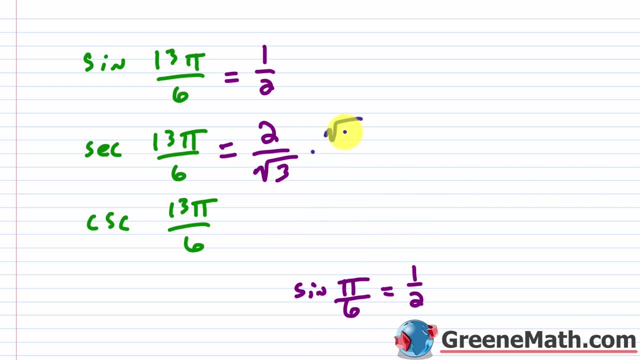 And so what I do here is just rationalize the denominator So times the square root of three over the square root of three. So this would give me two times the square root of three over three. Okay, Then, for my cosecant, I'm going to flip. I'm going to flip my sine, Right? So if 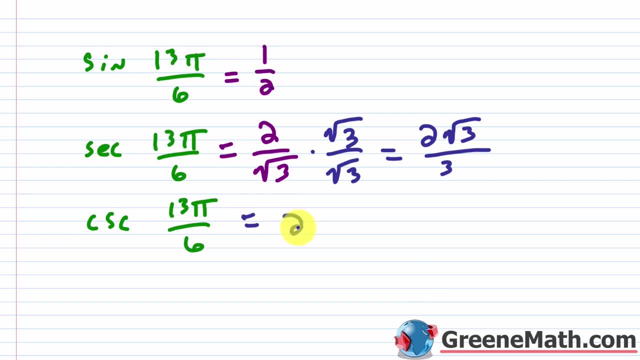 I flip that the reciprocal of one half is just going to be two. All right, let's just do one more example. So I'm going to look at the sine of: let's do negative 23 pi Over four. Let's also do the cosine of the same guy: negative 23 pi over four, And let me just kind 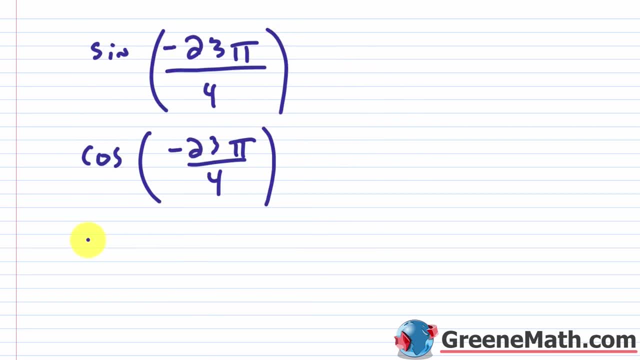 of move these up and out of the way. And then let's also do the cotangent, Okay, The cotangent of let's do negative 23 pi over four. Okay. So now that we have a negative angle, remember, if you have a negative angle, you want to do the same thing, You want to find a coterminal angle. 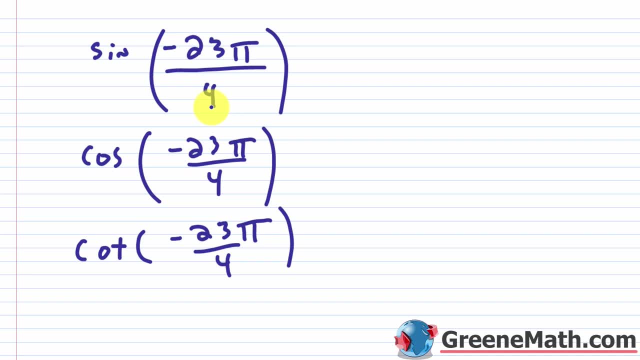 in terms of radians. So what I'm going to do is I'm going to add two pi radians until I get into that range. So let's go to a fresh sheet and say I have negative 23 pi over four If I add two pi radians. well, two pi. 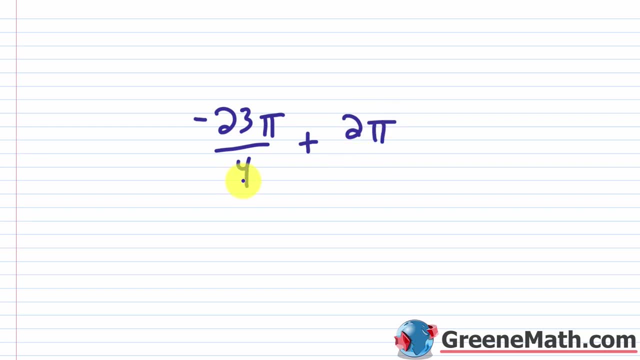 to this again. I want a common denominator, So I would multiply this by four over four, So you could say: this is eight, Okay, Eight, and then four down here, Okay, So eight pi over four now. So would this get me where I need to be? Okay, So I'm going to add two pi radians until I get into. 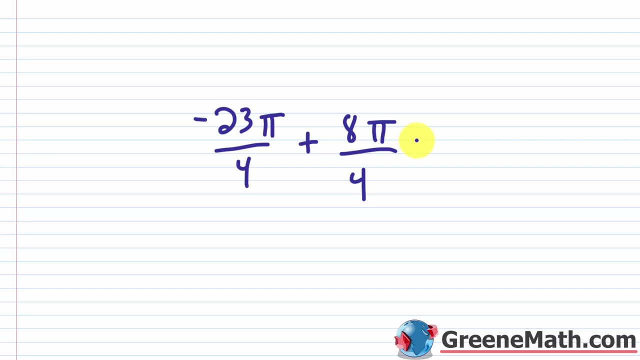 No, So I can add another two pi radians. So I can add another eight pi over four. Again, all I'm looking for is for this guy to not be negative. right, It's got to be between zero and two pi, Okay, So if I add eight plus eight, that's 16.. That's not going to get me there, So 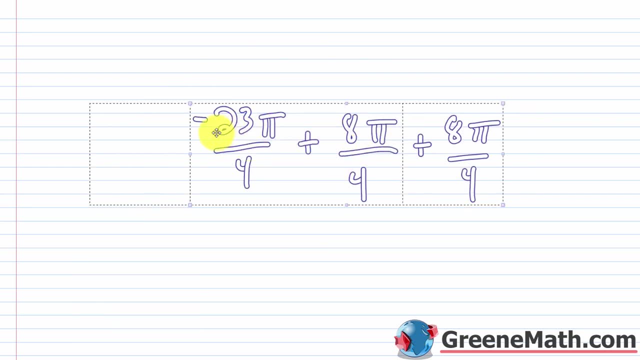 I need to add another one. So let me kind of scooch this down. So let me add another eight pi over four, and that would get me there, Right? So eight plus eight plus eight would be 24, 24 minus 24.. So that would get me there. So I'm going to add another eight pi over four, And that 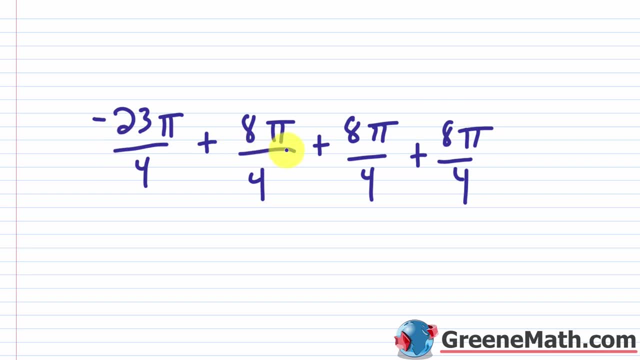 would be one, Okay, And you can do this with one common denominator and say that you have negative 23 pi, plus again eight plus eight plus eight is 24.. So this would be 24 pi all over the common denominator of four. So this would end up giving me one pi, or just pi over four, in terms of 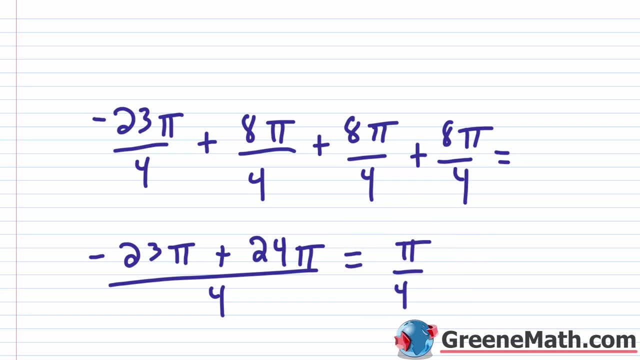 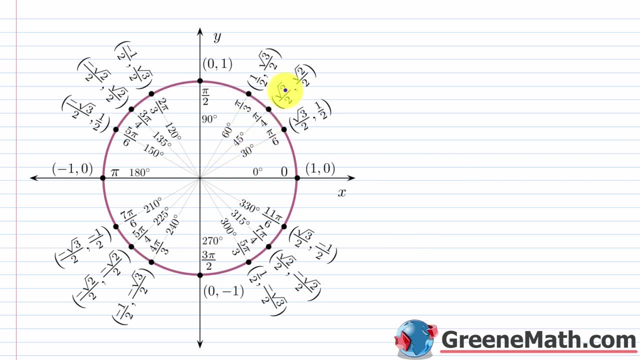 radians. So this is my coterminal angle. So let's go find that guy. So on the unit circle, if I look at pi over four in terms of radians, or 45 degrees in terms of degrees, I can get the square root of two over two and then square root of two over two. So that's really easy. 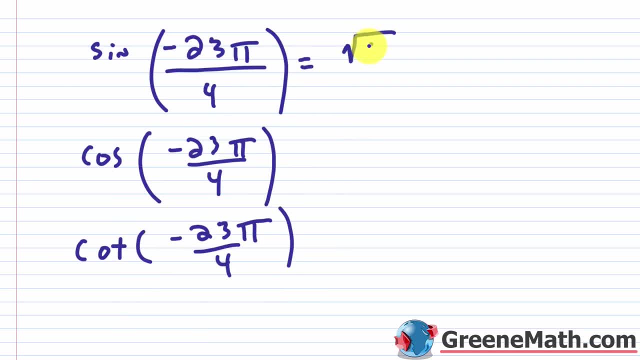 to remember. So I know, the sine of this guy would be the square root of two over two. Okay, And the cosine of this guy would be the square root of two over two. Now, what about the cotangent? Remember, the tangent is sine divided by cosine. Well, the cotangent, you flip that, it's the cosine. 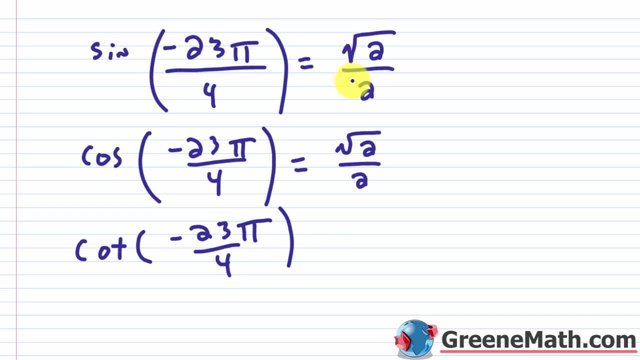 divided by the sine, But in this case I have the same thing divided by itself. Either way you go, either for the tangent or for the cotangent, it's the same thing. So in each case, this is just going to be equal to one In this lesson. 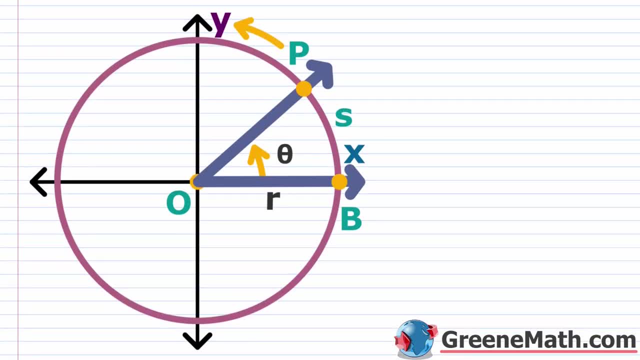 we want to talk about linear and angular speed. So previously we talked about how to solve motion word problems using our distance formula. So that's, the D for distance is equal to R, which is the rate of speed, times T, which is the amount of time traveled. So we're going to relate. 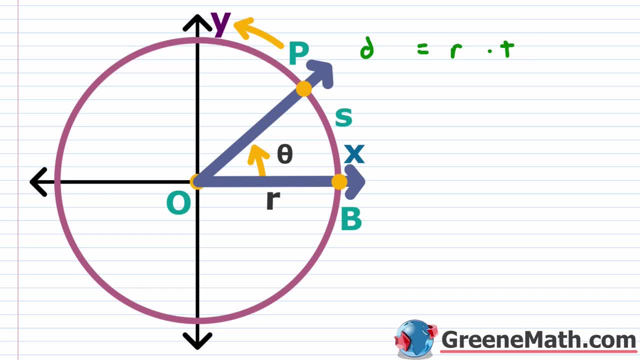 this formula to linear speed, which we'll talk about in a moment. Basically, if we know our rate of speed and we know our time traveled, we know our distance. So we're going to relate this formula to our distance. So, for example, if I plugged in 80 miles per hour here and I plugged in, let's say, 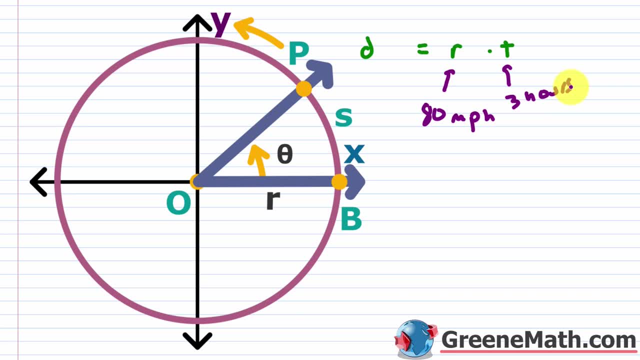 three hours here. what would be my distance traveled? So we sit in a car, we're moving at 80 miles per hour. We do this for three hours. We know that we would do 80 times three or 240. This would be 240 miles. Okay, So this is the distance traveled. Now let's suppose we didn't. 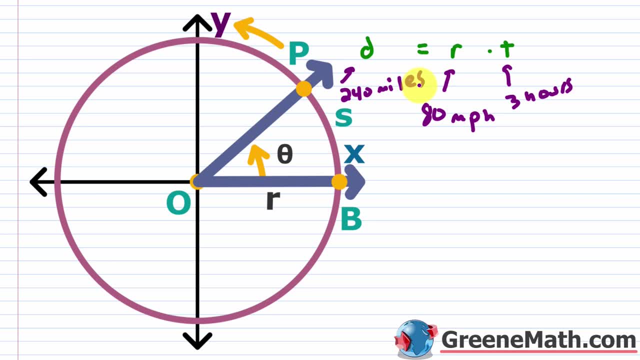 know the rate of speed, but we did know the distance traveled and we knew the amount of time traveled. So we're going to relate this formula to our distance traveled. So we're going to relate this formula to our distance traveled. So we're going to relate this formula to our distance traveled. 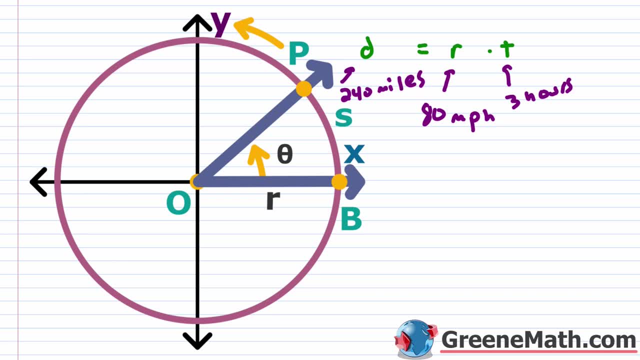 So now what I could do is I could solve this formula If I had D is equal to R times T. I could solve it for R right And I could plug in and find out what R is. So this would give me. 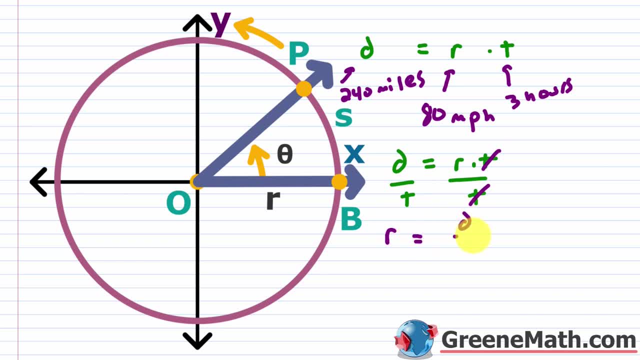 this cancels. the rate of speed is equal to the distance traveled divided by the amount of time it takes to travel that distance. So let's erase this and let's think about these numbers again. just as a simple example, So suppose my distance again is 240, and this is going to be in terms of 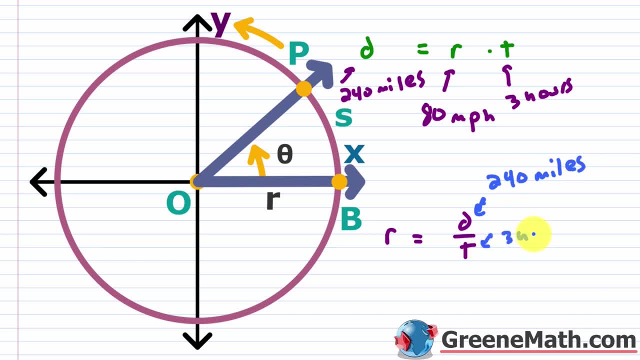 miles. Let's suppose my distance traveled is 240, and this is going to be in terms of miles. Let's suppose my time again is three hours. So now, if I have this information given, what's my rate of speed? Again, 240 divided by three would give me 80,. okay, And in terms of 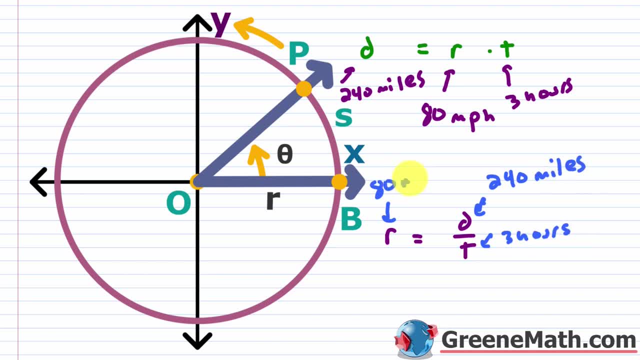 units miles and then hours. you'd have miles per hour, So miles per hour, okay. So very easy to understand this concept. Just think about all the times that you've traveled on a road trip and you've calculated how far you're going to be at what time, okay. So let's erase this, and I'm 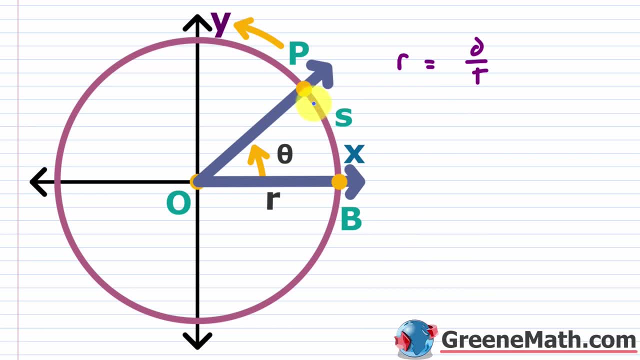 going to use linear speed now. So for linear speed, let's look at our little diagram here. I want you to suppose that some point P- okay, So this is my point P- It's going to move at a constant speed along a circle with this radius of R, okay, And with a center of O, okay. So the 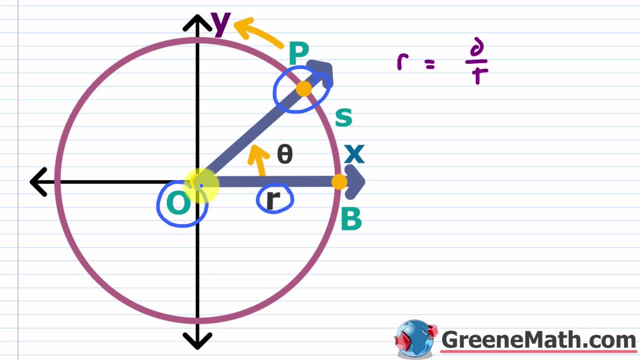 measure of how fast the position of P is changing is known as the linear speed. okay, So instead of R, we're going to use V. okay, for velocity, And instead of D now, because we're traveling along a circle. remember, when you think about the distance or the length, that you're traveling on a 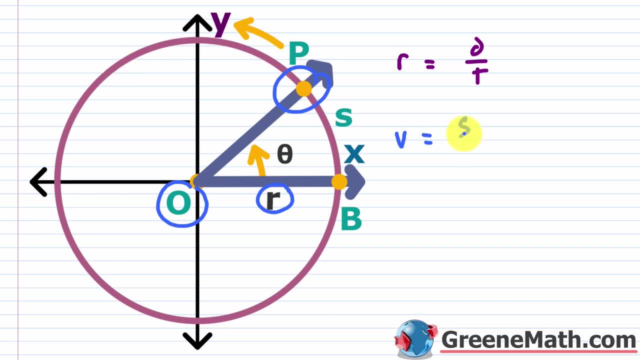 circle. this is the arc length, right? So we use S for this. So now I'm going to have S over T, okay, So that's how these two guys are related. Instead of R, we use V for velocity Instead of. 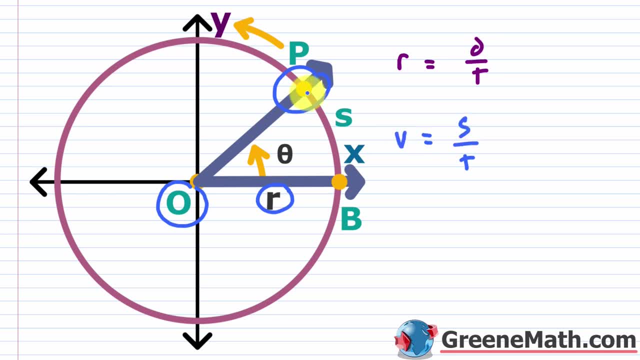 D for distance. we're going to use S for the arc length that's traced by this point P at the time T. To put this in more simple terms, the linear speed is just the speed at which a point on the outside of some object travels in a circular path around the center of that object. So that's the 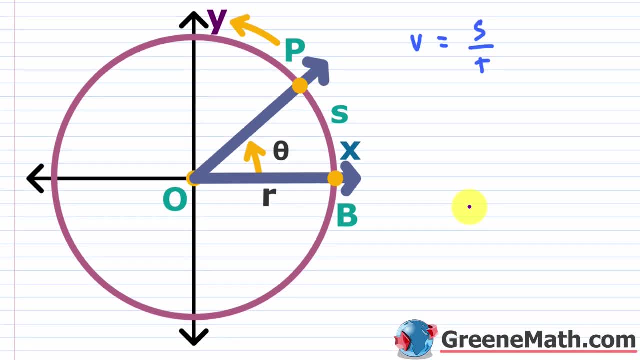 object. Now, when we talk about angular speed, we're talking about how fast the measure of the angle is changing. So again, if I think about this point here, P right. So this is the terminal side of the angle, P OB. If I'm rotating P around this circle, the measure of the angle is changing. 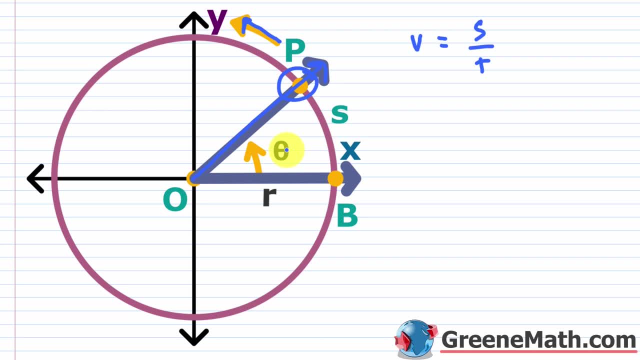 okay, So how fast the measure of that angle changes? that's our angular speed. okay, So this is given by the formula You're going to use, this letter omega. okay, And I'm terrible at it, but this is the Greek letter omega and it's equal to theta. okay, Which is the angle measure. 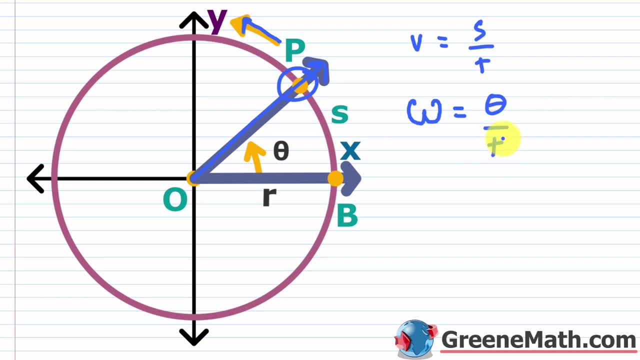 in radians divided by T, which is your time Now. there's one more thing I want to talk about before we get to the problems. You might want to make a little substitution, okay, Based on what you're given in the problem. you might want to make a little substitution here And instead of saying 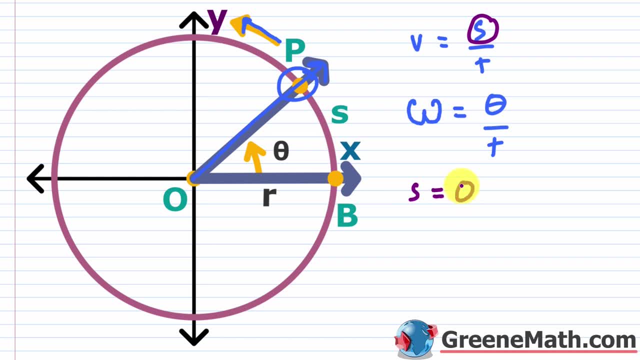 ask the arc length. remember the arc length asked is equal to your theta okay, Your angle theta okay. So if we plug in there we could say V is equal to you would have your theta times R okay over T. Now we know from fractions that I could really rewrite this as R times your theta over T. 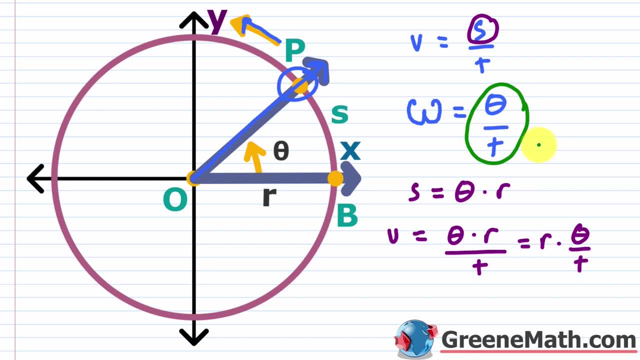 So now we can make a little substitution, because theta over T- okay, is this guy right here? okay, It's the Greek letter omega, which again is our angular speed. So I can put this as my angular speed. So the linear velocity or the linear speed, however your book says it is going to be equal to. 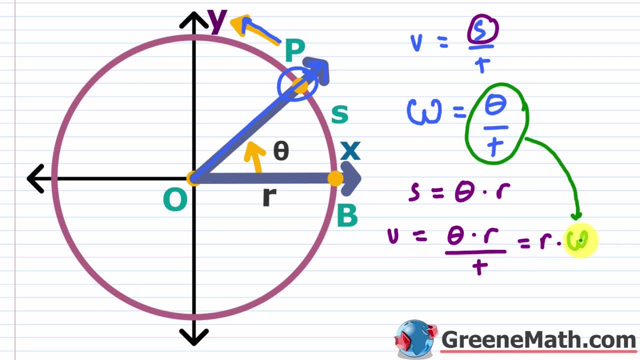 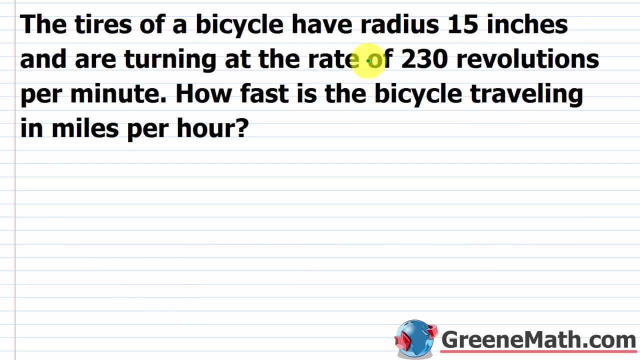 the length, of your radius times, your angular speed. So let's go ahead and look at an example. So the tires of a bicycle have radius 15 inches and are turning at the rate of 230 revolutions per minute. How fast is the bicycle traveling in miles per hour? Okay, so the first thing you want. 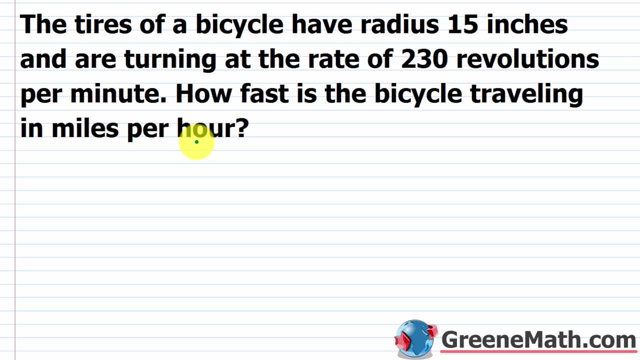 to do for a problem like this is calculate the angular speed. So again, I'm going to try to make this a little bit easier. okay, This is equal to, again, theta over T. okay, So the first thing you might notice is that you're given this rate here of 230 revolutions per minute. okay, When you think, 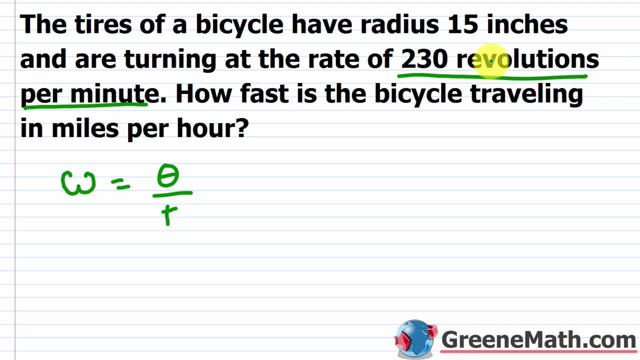 about one revolution. it's one complete circle, or 360 degrees, or 2 pi radians. Since we're working with radians here, we want to put 2 pi up here. okay, This is one complete revolution or one circle. We have 230 of these. 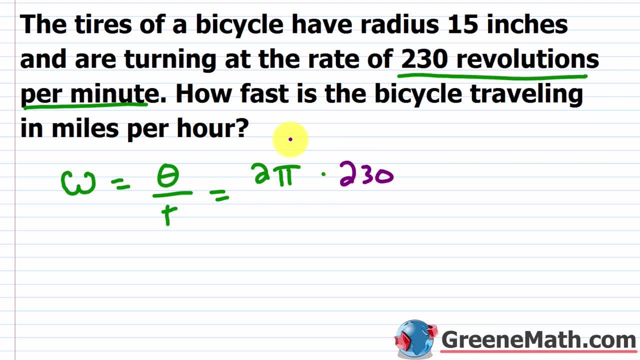 So I'm just going to multiply this by 230, okay. So again, this is one complete circle, or one complete revolution, or one complete rotation, however you want to think about that. okay, So it's 2 pi, okay, or 360 degrees, if you want to relate it back to degrees, Then we have 230 of 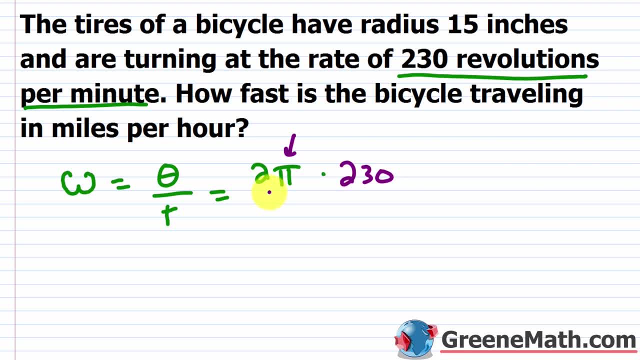 these guys. so that's why I'm multiplying by 230.. Now I'm going to divide this by the time is given as per minute, So per minute means one minute there. okay, So this is in terms of radians, so you can write this as radians. okay, right here. So this is 2 pi times 230, or you could say: 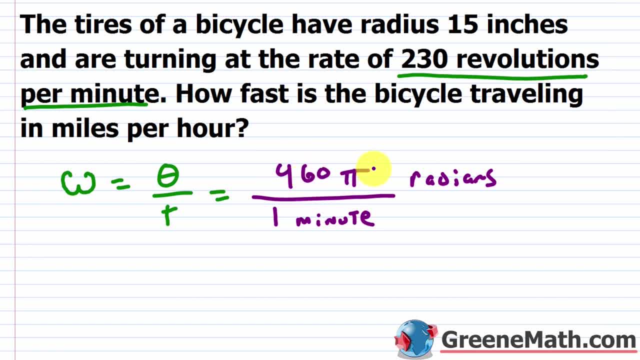 460, 460 pi radians per minute. Now the next thing we want to do is think about the time units that we want. It's going to ask for this in terms of miles per hour. We have radians per minute, okay. 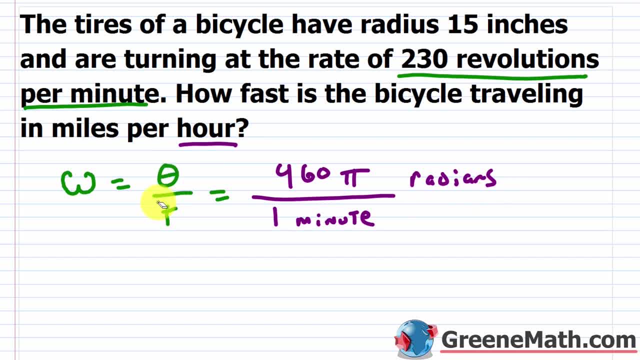 So we want to convert this to radians per hour. So let me erase this so we have a little bit more room to work, because this can get quite messy. So let's move this down a little bit and I want to multiply this now by what I want: hours in the. 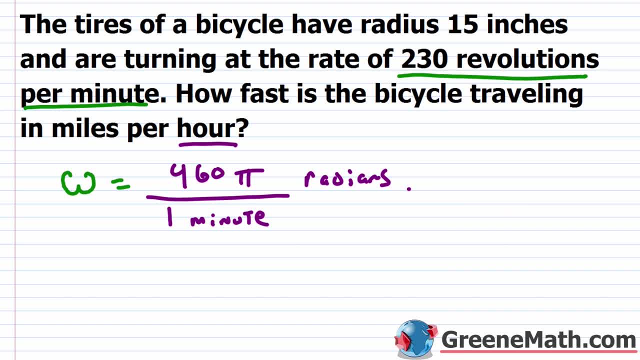 denominator. I want one single hour because I want per hour. okay, So if you always think about what you want, go ahead and put that there first, and then how do I get there? I want minutes to cancel. What's the relationship between hours and minutes? Well, 60 minutes. 60 minutes is equal to one hour. 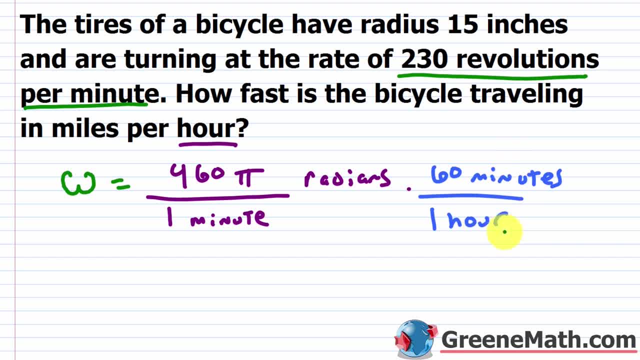 okay, So now this is basically equal to one. okay, So what I can do is I can cancel this with this and I'm left with the units that I want in my denominator. So let's go ahead and multiply 460 by 60,, which is 27,600.. Don't forget the pi there. It's easy to forget it, Pi, and then you have. 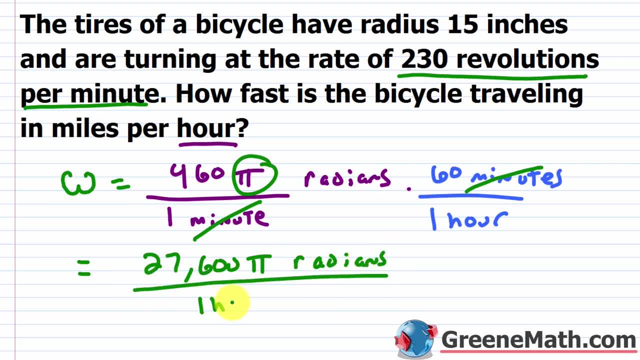 radians, okay, And then per one hour: okay. So that's your angular speed: 27,600 pi radians per hour, okay. So let's erase this. I don't need these intermediaries, I don't need steps anymore, and let's just bring this up here and I'm just going to say it's 27,600. 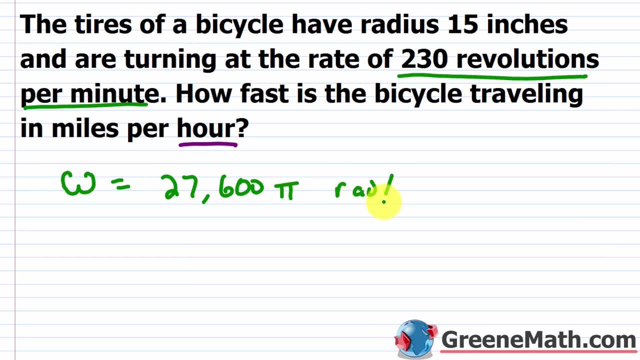 pi, and then I'll put radians per hour. okay, I'm just going to abbreviate there. Now let's think about now the linear speed: okay, in terms of miles per hour. So how are we going to get this? 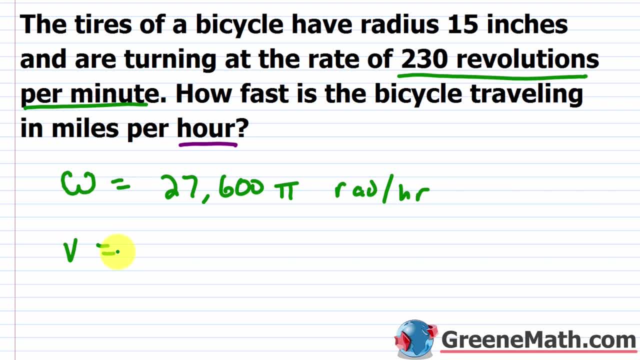 So v is your linear speed. Remember the formula we looked at when we plugged in here? We said that we could do the radius times, the angular speed. So if we come back down here, the angular speed, I'm going to put 27,600 pi, okay, And then you can. 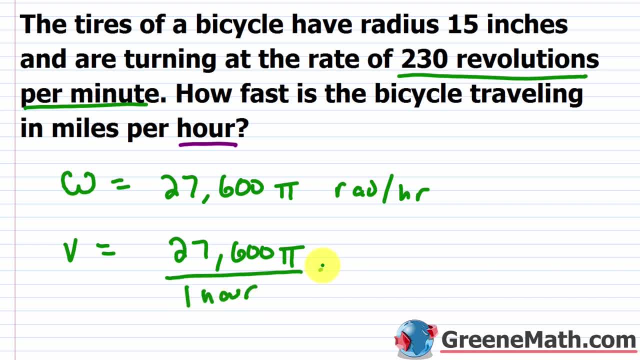 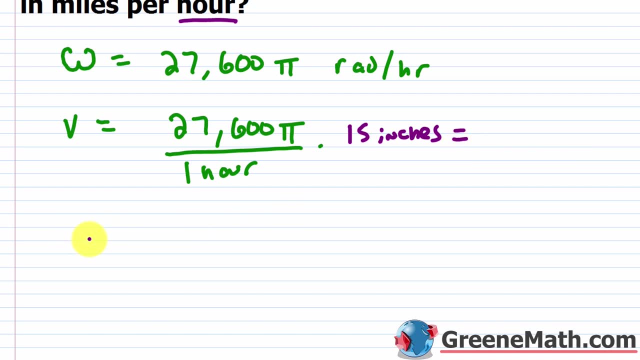 go per hour. Let's put this down here And then times: what's the radius? Well, the radius is going to be given to us here as 15 inches, So 15 inches right here. If I multiply this out, let me scroll down and get some room going. If I multiply this out, I'm going to get that. 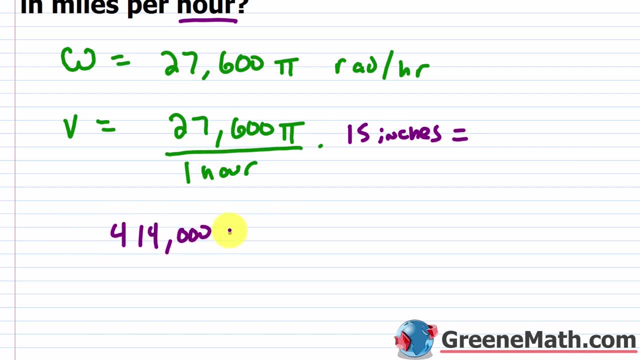 414,000 pi. Okay, and then we'll say inches per one hour, okay. This is not what I want, though, because I want it in terms of miles per hour and I have it in terms of inches per hour, okay, So I've got to. 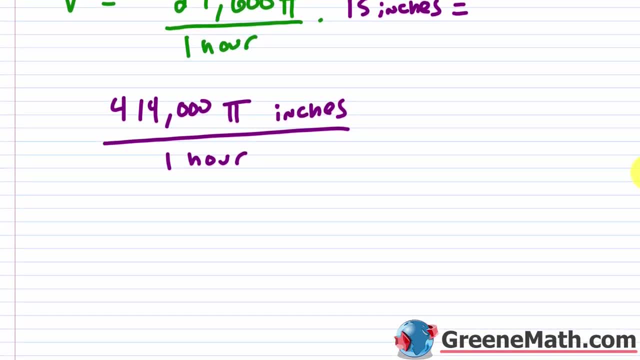 do another unit conversion and this is where these things get kind of tough. So if you know the relationship between inches and feet, 12 inches equals one foot and then you can convert from feet to yards and then from yards to miles. I'm going to shorten this up, So the relationship 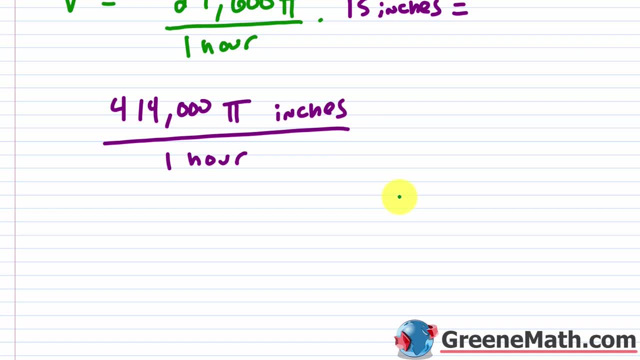 between inches and feet is 12 inches, and then from yards to miles, and then from yards to miles, and then from yards to miles, then from yards to miles. what's the value of 136 inches? Well, reach out and look at the analog range and that's going to be horizontal 가로. 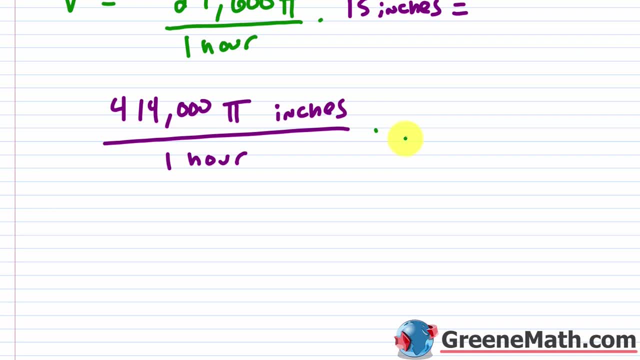 And in order to get 16 inches in miles, 33,360 inches is equal to one mile. So what I can do, I want inches to go away. So I'm going percent to a Kalau deviation and issued $, biting one, and then it's going to be 360 inches. Okay, I want that to go away. so what then? 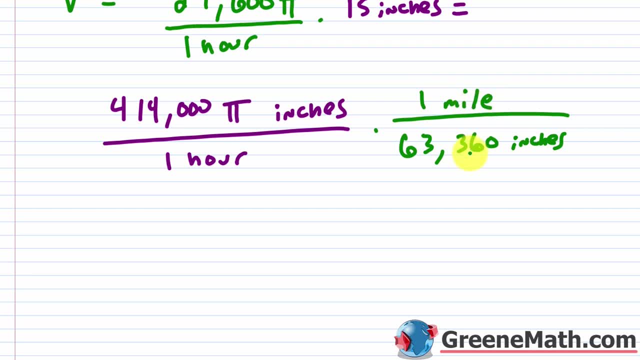 the denominator And we'll put one mile in the numerator. Again, one miles equal to 63,360 inches. So space is: If we're going to use teriablank aisle ID color, everything's an Excel FLM that has rec wagon- okay. So this would cancel this. So those units are gone. So now it's gonna. 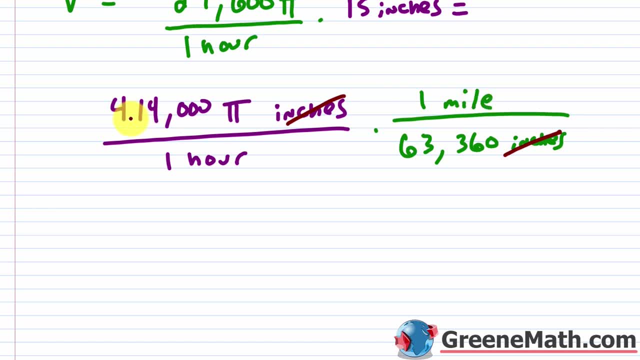 per hour, Okay. So what you'd want to do is really just take 414,000 pi, Okay, And then divide it by this number here, 63,360.. It's going to be an approximation, because you're going to get a. 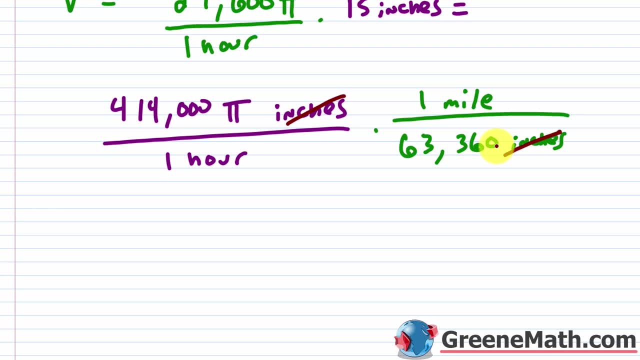 decimal number. But if you wanted to simplify this first, you could divide this by 720.. Okay, And you could divide this by 720 and that would give you 575, and this would be 88. Okay, So you can really write this as 575 pi miles, Okay, Per your 88 hours. But again, this is kind of useless. 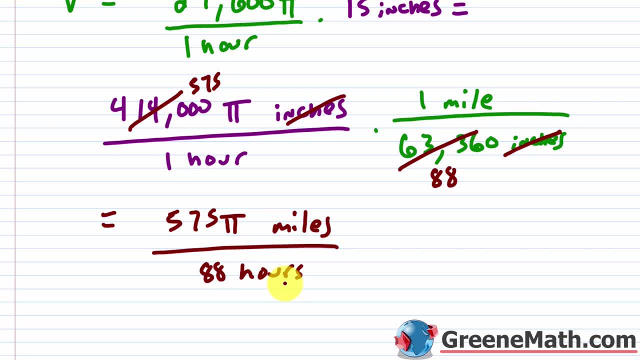 because we want miles per hour. So if you punch this up on a calculator, you could say that this is about 20.5.. This will be in terms of miles per hour. Okay, So that's our linear speed. So let me. 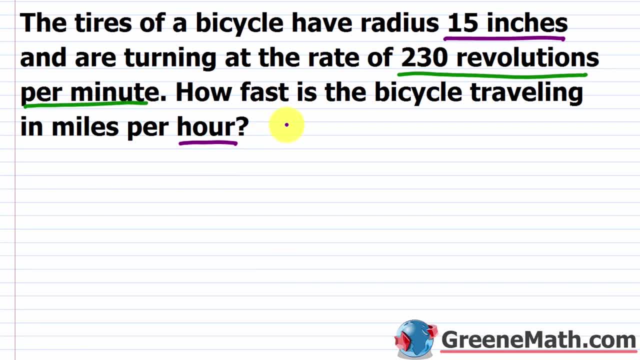 just erase all of this. So to answer this with a nice little sentence, I'll say: the bike. the bike is traveling at about because, again, this is an approximation 20.5.. And this is in terms of miles per hour. 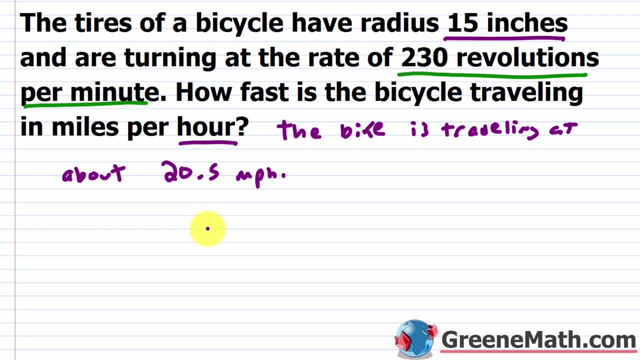 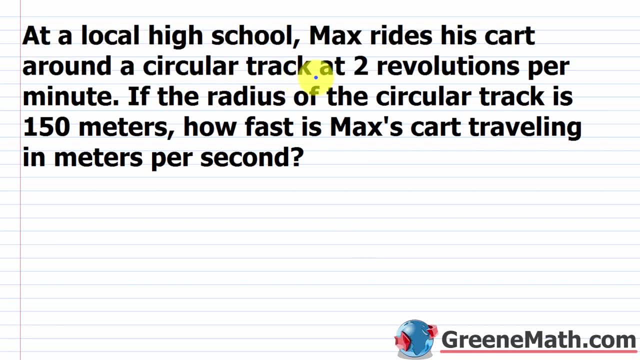 So the bike is traveling at about 20.5 miles per hour. All right, Let's take a look at one more problem. So at a local high school, Max rides his cart around a circular track at two revolutions per minute. If the radius of the circular track is two revolutions per minute, the bike will. 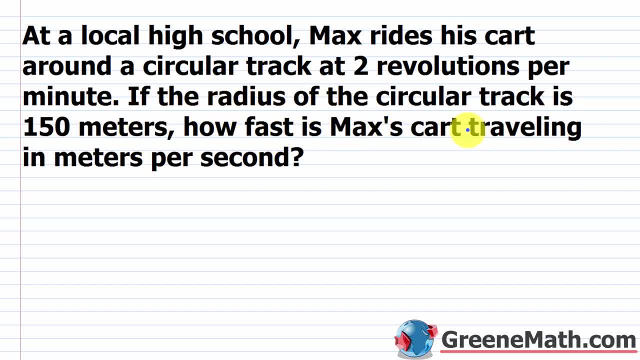 ride a circular track at 150 meters. How fast is Max's cart traveling in meters per second? Okay, So a similar setup. I'm going to use omega once again to say it's theta over t, right? So this is my. 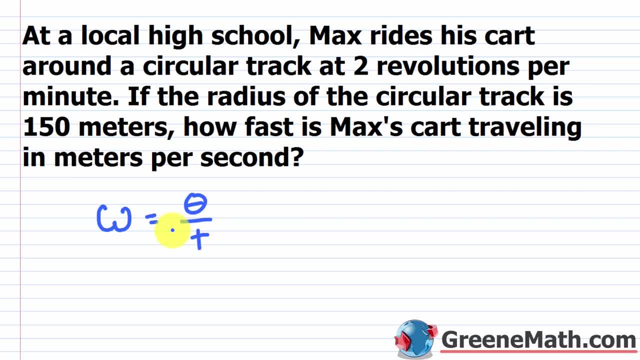 angular speed. So what is theta in this case? Well, we have two revolutions, and this is per minute. So down here this would be- let me put t as one minute and get that out of the way, And I'm just going to abbreviate it, For theta it's two times two pi, Again one revolutions per minute. 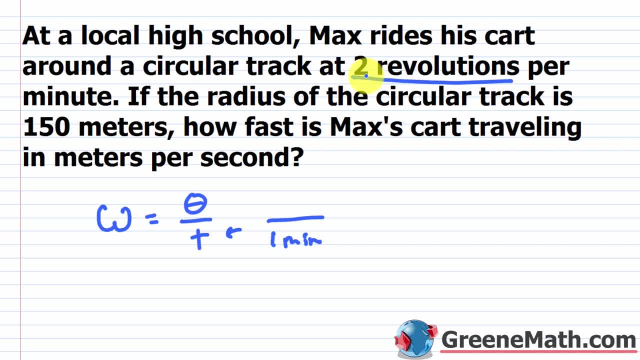 So this would be one revolution or one time completely around a circle is two pi radians, or 360 degrees. So you have two pi okay times. you've got two of these revolutions, So two. So this would be four pi, four pi radians. radians per minute. Okay, So that's your angular speed. Now we want. 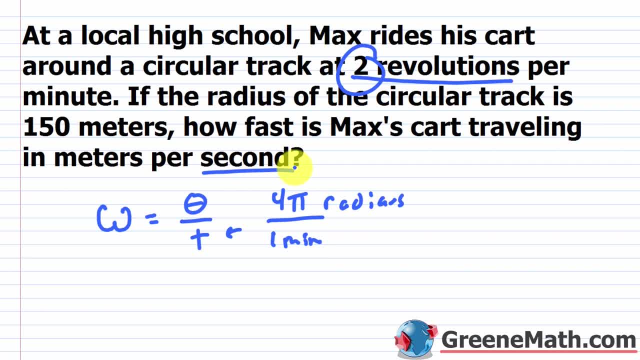 this in terms of seconds, but let's convert this in a moment because it's gonna be a little bit easier for us. We know that with the linear speed, okay, if we're trying to find out how fast Max's cart is traveling in meters per second, we're going to have to convert this in a moment. So 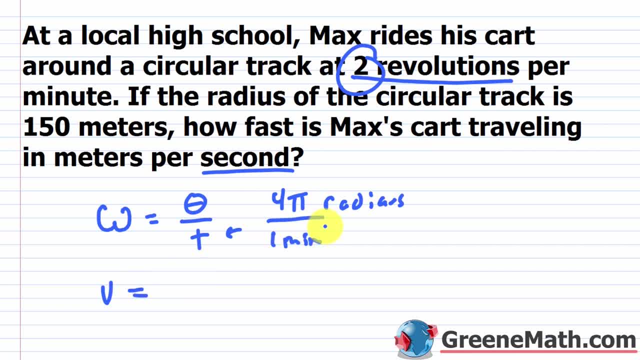 let's do that. So we have four pi over one minute times the radius. It tells us 150 meters. So it's 150 meters, Okay. And so let me scroll down and get some room going here. Okay, So four times 150,. 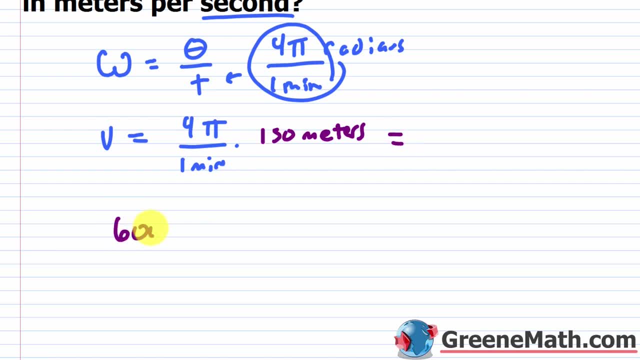 we know is 600. Okay, So let's do that, So let's do that. So we have four pi over one minute times 600.. So this ends up being 600 pi meters, Okay, Per one minute. So the last thing we want to do is: 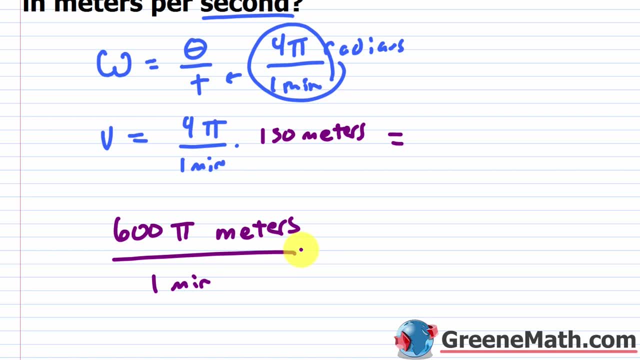 get this in terms of seconds, Okay, And the reason I waited here is because you have to divide by 60, and 600 divided by 60 is pretty easy to do, Okay, So that's why I waited, So you can multiply this. 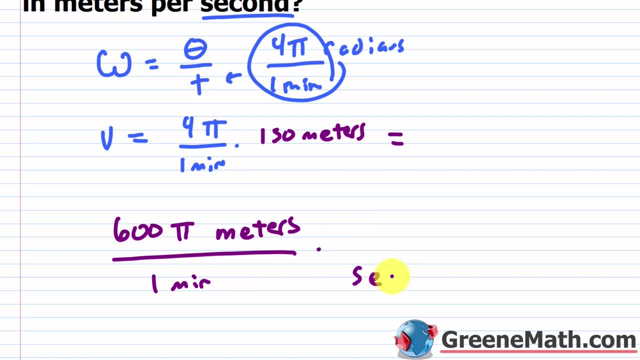 now by: I want seconds in the denominator because I want it as per second And there's 60 seconds in one minute. Let me slide this down. I kind of ran over a little bit. Let me slide this down and I'll put one minute up here so that it will cancel Again. you want to? 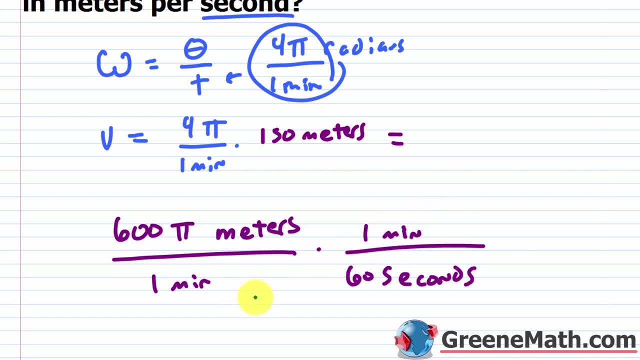 and let me abbreviate this so that it's consistent. You want to put these across from each other again, so they cancel. So this will cancel with this, And I'm just left with seconds. now, right, I'll have meters per second. So 600 divided by 60 is going to give me 10. So this would be 10 pi. 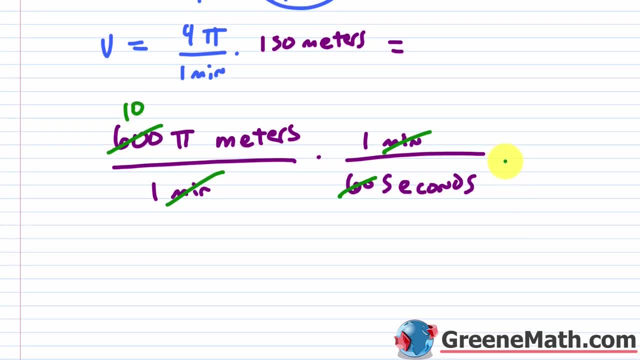 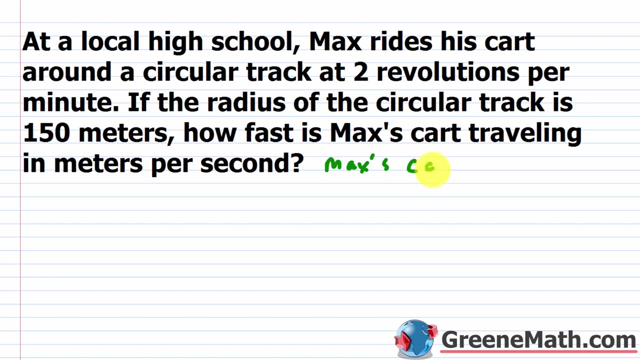 meters per second, Or you could say it's about. you could say it's about 31.4 meters. Okay, Meters per second, Okay. So to answer this little word problem, I'll say that Max's cart, Max's cart is traveling. 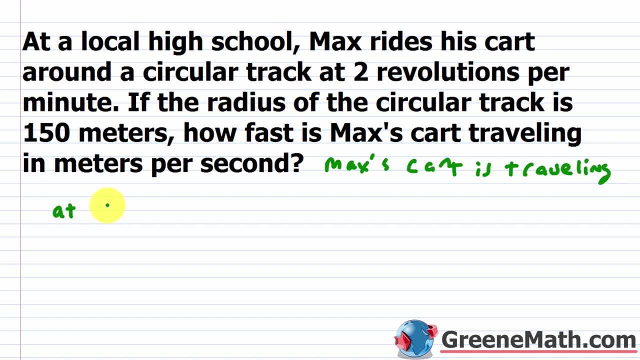 at about- again, it's an approximation- 31.4 meters per second. Okay, So Max's cart is traveling at about 31.4 meters per second. Okay, So Max's cart is traveling at about 31.4 meters per second. 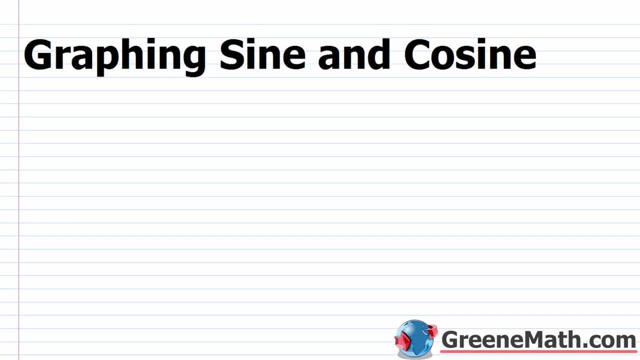 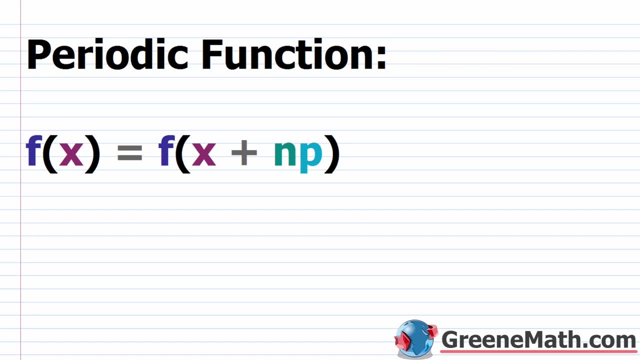 In this lesson we want to talk about graphing sine and cosine. All right, So to start out the lesson, I'm going to talk about something called a periodic function. So when we think about sine and cosine, these guys are called a periodic function because their values repeat in a 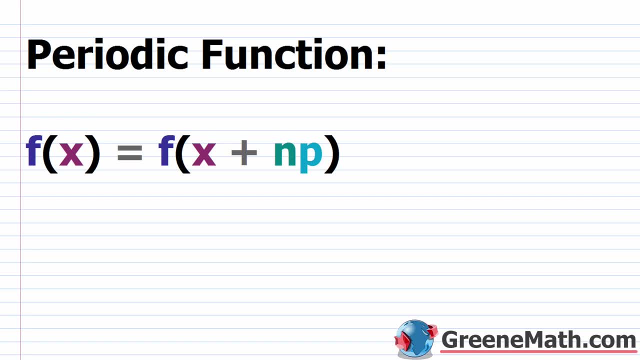 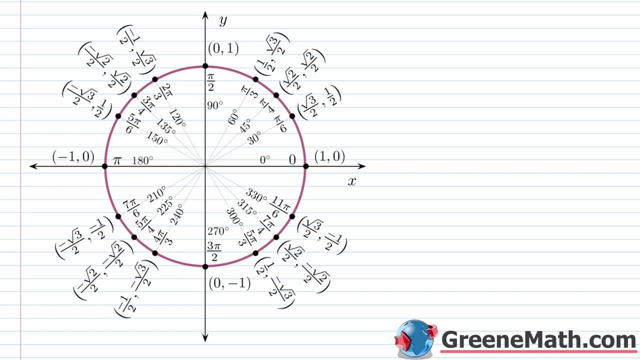 regular pattern. So to see what I mean by that, let's revisit the unit circle from the last section, So from our unit circle. what we see here is that as we travel around we're going to see around our unit circle. So in other words, if I start here, let's say I make a counterclockwise. 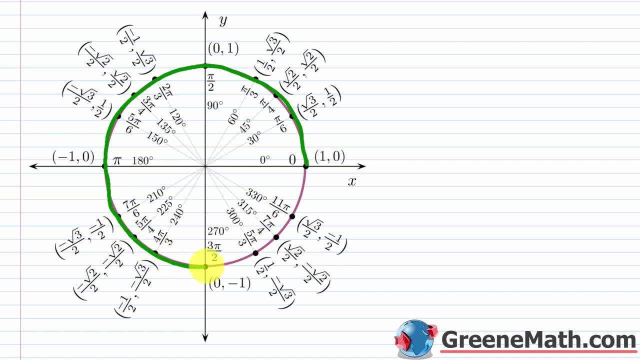 rotation. Okay, So a positive angle measure and I do one full rotation. Well, that's going to be an angle measure of two pi. We already know that. Okay, But as I continue past two pi, so let's say I created an angle that was greater than that, So I keep going around. Okay, So let's say I make an 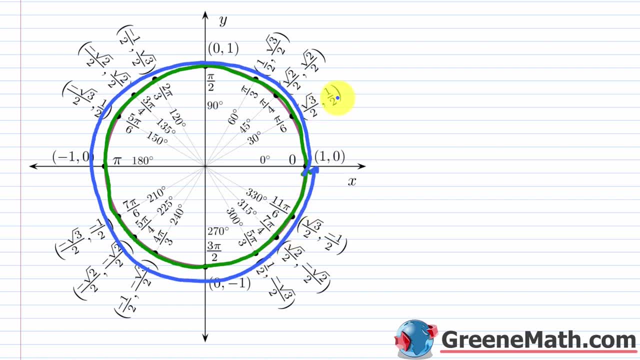 angle that's four pi, So two full rotations. What's happening is these values for sine and cosine are going to repeat. So let's say I make an angle that's four pi, So two full rotations. What's happening is these values for sine and cosine are going to repeat themselves. Okay, So anything? 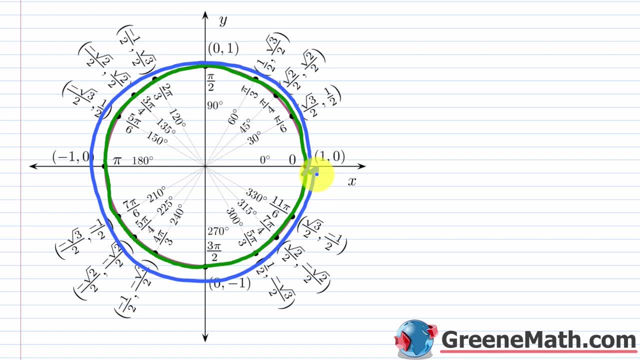 past two pi. So when we talk about two pi for sine and cosine, this is going to be known as our period. It's the smallest possible positive value for where these function values. okay, these values for sine and cosine are going to repeat themselves. Okay, Let's think about this with a simple little 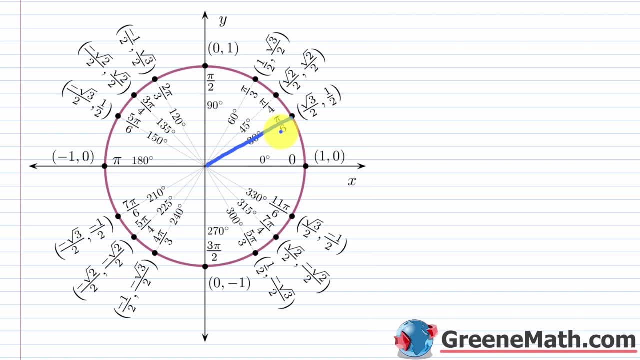 example, Let's say, I think about this angle measure here, which is pi over six or 30 degrees. I know that the sine of pi over six is given by the y value of that point right there. Okay, So this is equal to: 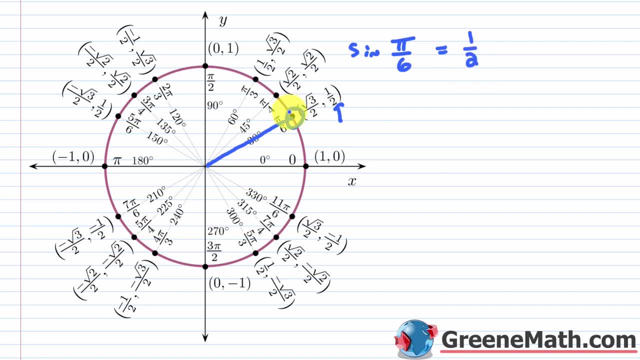 one half, Okay. But also if I was to rotate around another two pi, okay, so another two pi. I'm going to get back to that same point right there. Okay. So I have a coterminal angle and my sine value is going to be the same. So, in other words, if I said the sine, 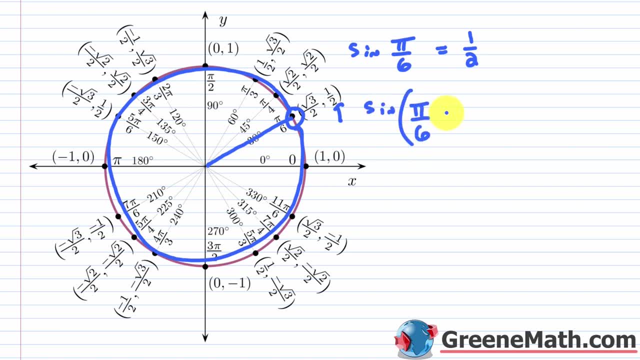 of pi. let me use parentheses here. pi over six plus another full rotation would be two pi. Let's go ahead and write that. Let's say you write that as 12 pi over six, So we can have a common denominator. This is going to be equal to a half as well. Okay, If I add these up, pi plus 12 pi is 13 pi. 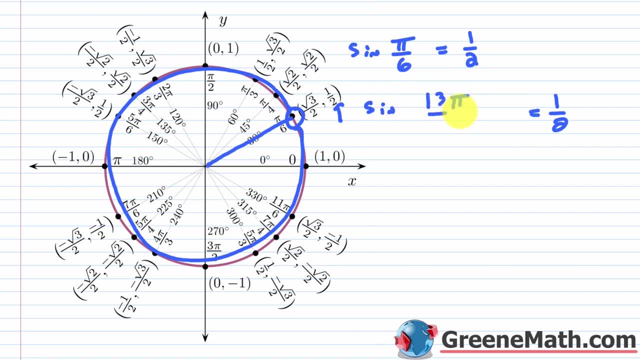 So this is 13 pi over six. Okay, This is 13 pi over six. If you punch this into your calculator, you'll see that you get the same value either way And you can keep going around another two pi, or you can go the other way. You can go clockwise two pi. So basically, as you're adding these, 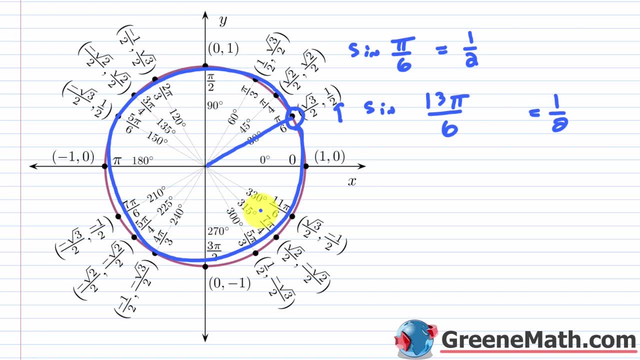 multiples of two pi, you're getting these coterminal angles And so your sine values are the same And also your cosine values are the same. So you're getting the sine values are the same And also your cosine values are the same. So if you add these up, you're getting the cosine values are the same. 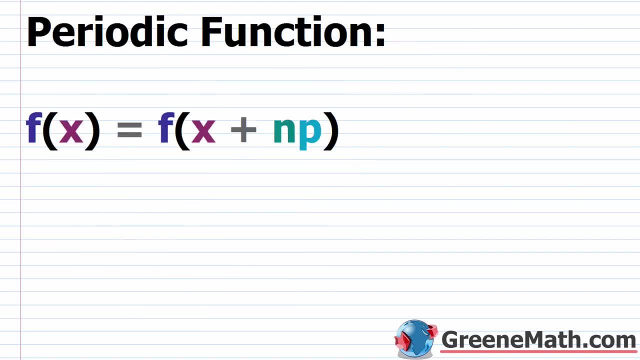 the same. so if we go back up to our little definition of a periodic function, you see we have f of x. x is just some member of the domain. in the case of sine or cosine it would be any real number. this is equal to f of. you have that same x value plus n, which is some integer times p, which. 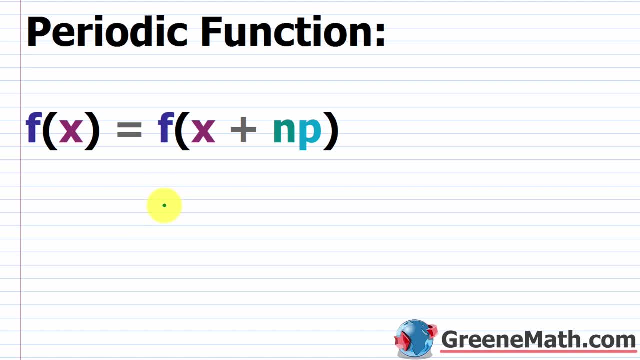 is going to be our period, which in this case, is going to be 2 pi. okay, so i could say something like the sine of x and i could say, really, this is equal to the sine of- i'll say that same x value plus some integer n times the period p, which is 2 pi. okay, this is something that is very. 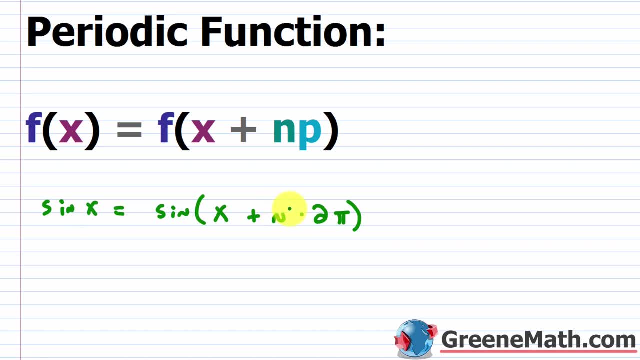 important to write down. we're going to use this not only in this section but also when we solve trigonometric equations. so then we could say: the cosine of x is equal to the cosine of. you have your same value for x plus your n times your 2 pi. okay, in our example, 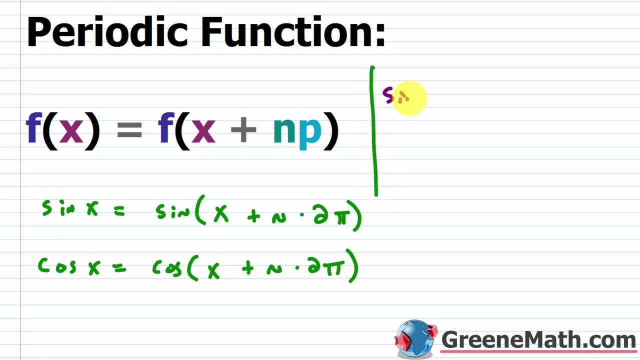 we saw- let me write this off to the side- that the sine of basically the pi over 6 was equal to the sine of. we had pi over 6 again. okay, and then what we did was we added just 2 pi. right, our n was 1, but really you could put n times. let me screw this down because it's going to run out of room. 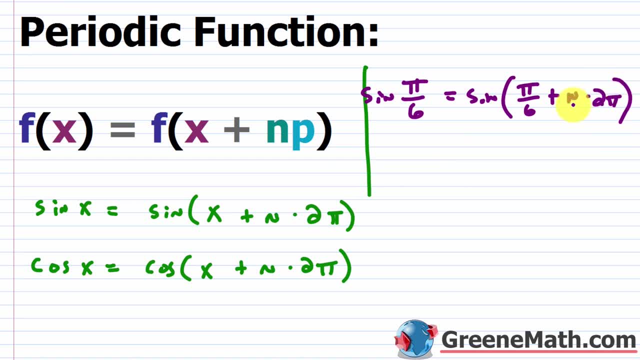 n times your 2 pi. okay, so you can plug in anything for n as long as it's an integer, and this statement would be true. you would basically get one half on the left and one half on the right after you evaluate. okay, before we move any further, i want to clear up something that is a common 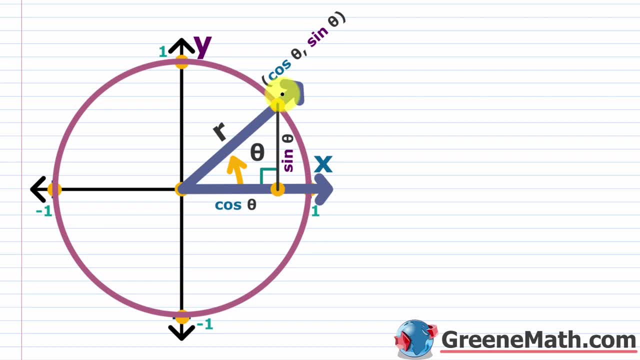 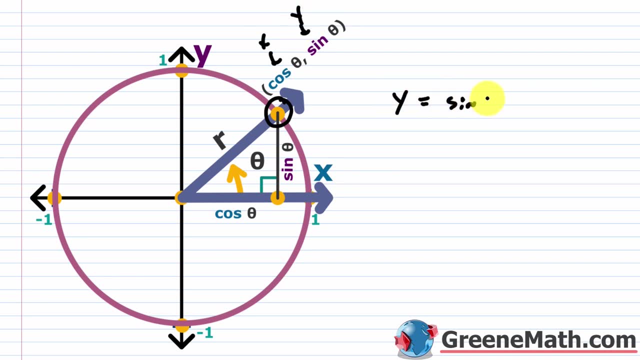 source of confusion, and that is what to do with this point right here, okay, which contains an x value and a y value. when you're working with something like y equals the sine of x or y equals the cosine of x, which we're going to get to in a moment. let me just erase this. okay, we'll build up. 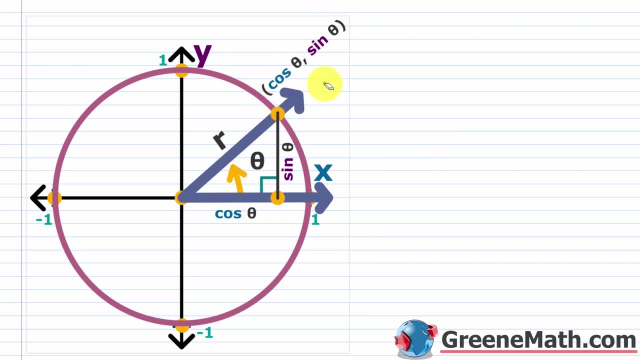 to what we need to do. okay, let me actually erase this. i want to show you again where things come from. even though we talked about in the last section, we have a unit circle here. okay, so that means the radius is 1. okay, so this r value here, or this. 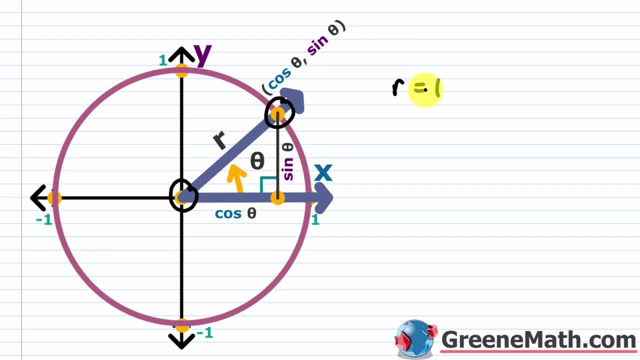 distance from right here to right here is 1. okay, you can see that from here, which is the origin, 0 comma 0, to here, which is 1 comma 0, that's 1. from here to here is 1. from here to here is 1 from. 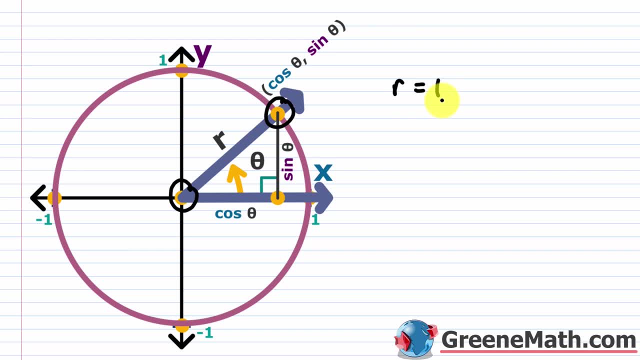 here to here is 1. so we see the radius is 1. now, if i go back to my definition of cosine of theta and sine of theta, again, if i have a point on the terminal side, well then the cosine of theta is given as x over r and the sine of theta is given as y over r. well, here my r value is 1. 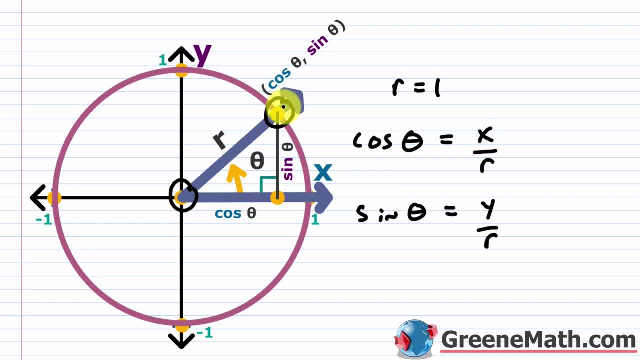 so the cosine of theta is exactly equal to x or the x coordinate from that point. so this is exactly equal to x. for the sine of theta again, y over r, r is 1, so this guy is exactly equal to the y coordinate from that point. so it's really important to understand that when i grab this. 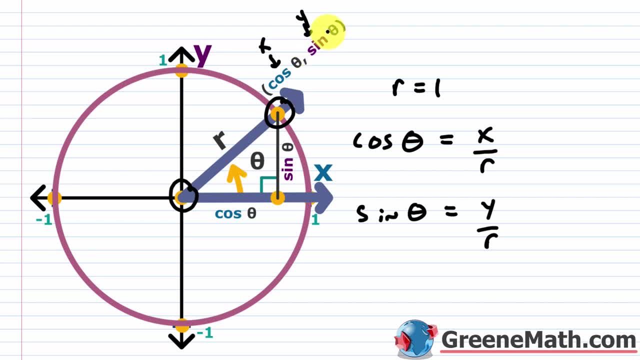 x value, it's the cosine of theta. when i grab this y value, it's the sine of theta, okay, so Okay, Now we move on and we introduced this S now instead of theta. Okay, That further complicated things. The reason we're using this is so that we can have real numbers as our domains for the. 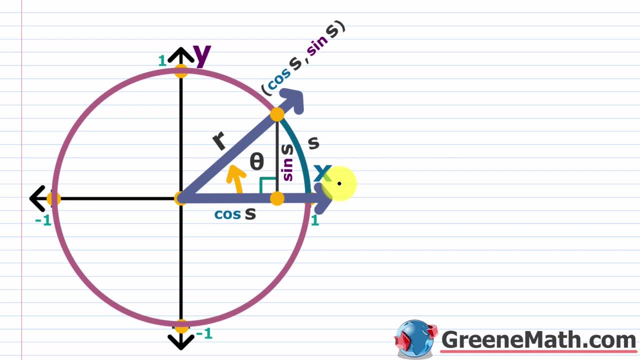 trigonometric functions. right, We started to call these guys circular functions. So S here is the arc length of the intercepted angle. Okay, So S is exactly equal to theta. Okay, So now we can say that for this point right here, the X value is the cosine of S. Okay, This arc length here. 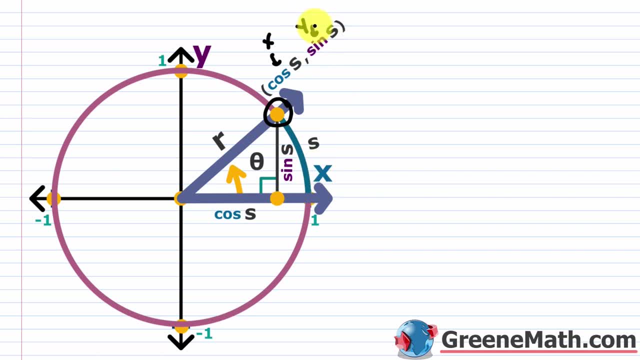 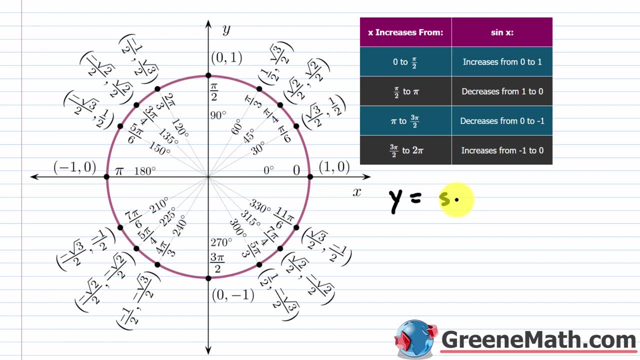 and then the sine of S is going to be Y. Okay, So that's all we really need to know. When we come back to our little unit circle and we think about something like Y is equal to the sine of X, or let's say, Y is equal to the cosine of X, It's important to know what's going on. 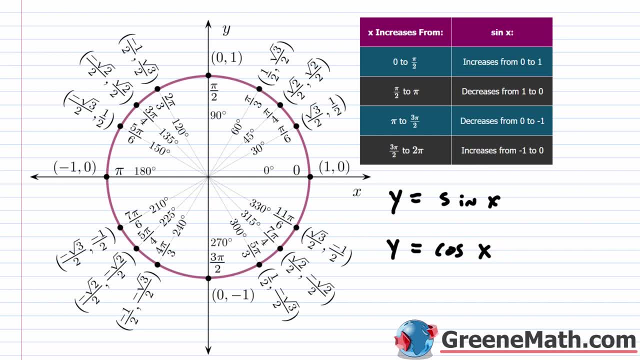 what you're plugging in for X and what you expect as an output for Y. We are plugging in angle measures here, typically in radians, for X and we are getting sine values out for Y, Okay, Okay. So in other words, if I look at- let's say this point right here- I am not taking this as the X. 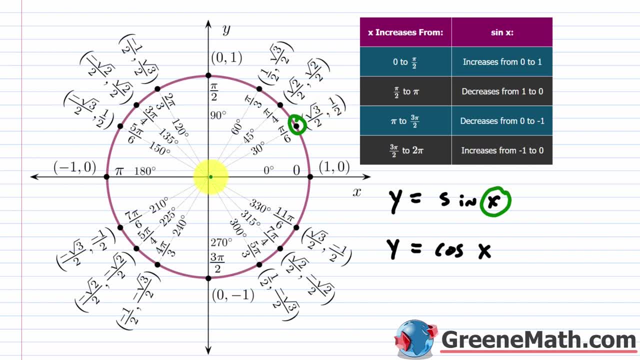 value and this is the Y value. That is not how that works. I want the angle. Okay, So pi over six, In other words. let me erase this for a moment. If I said Y is equal to the sine of pi over six, what's the Y value? Well, the sine of pi over six is given by this Y value. here for this, 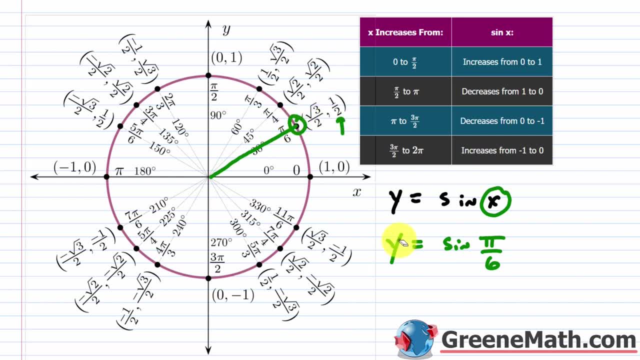 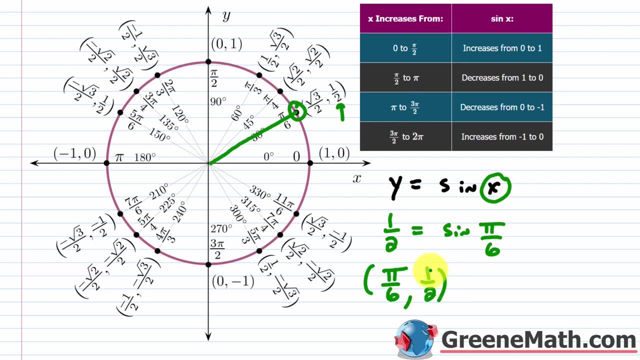 point right. The Y coordinate from that point, which is one half. So this guy right here would be one half. In other words, a point would be pi over six, comma one half. Another one would be: let's say I did. 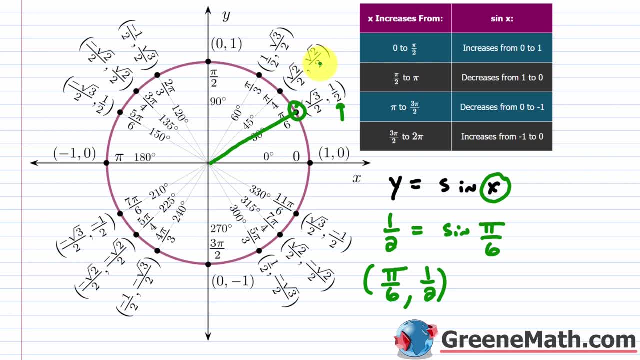 pi over four, Well, the sine value would be square root of two over two. So another one would be pi over four, comma, square root of two over two. Okay, You can continue making points like this to sketch your graph of sine. I'm going to show you a better way in a moment. 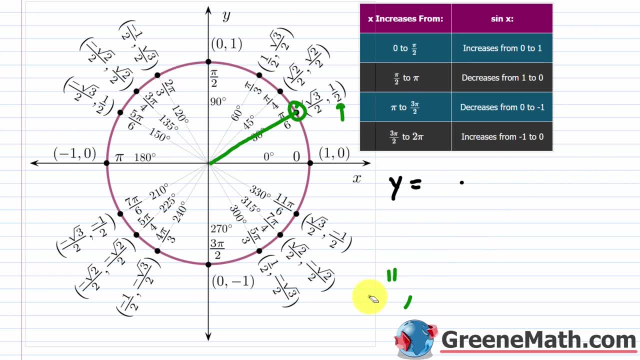 but for right now I just want to make sure that's clear for you. Okay, If I did a few with cosine just really quickly. So Y equals the cosine of X. Again, if I plugged in pi over six, I would get the Y of cosine. So Y equals the cosine of X Again if I plugged in pi over six. 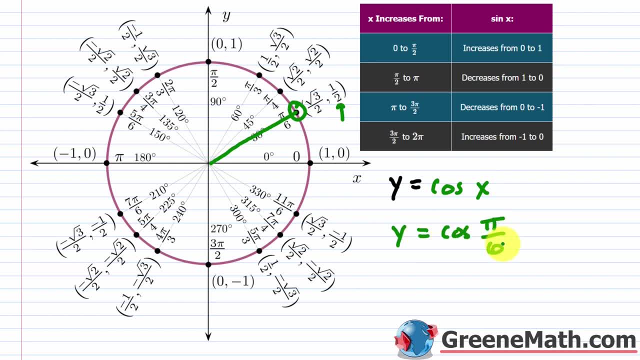 so Y equals cosine of pi over six. Well, what is the cosine of pi over six? I'm not looking at the Y value now, I'm looking at the X value for this point. Okay, It's square root of three over two. 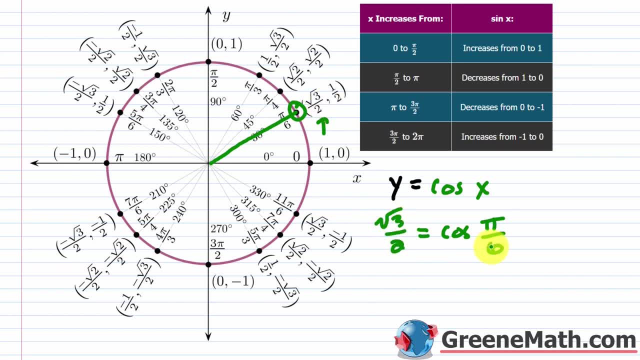 So this would be square root of three over two, And so the ordered pair there would be pi over six, comma, square root of three over two. Okay, So it's very important that this is clear for you in terms of what you're plugging in for X and what your output is for Y. Now, with that being said, 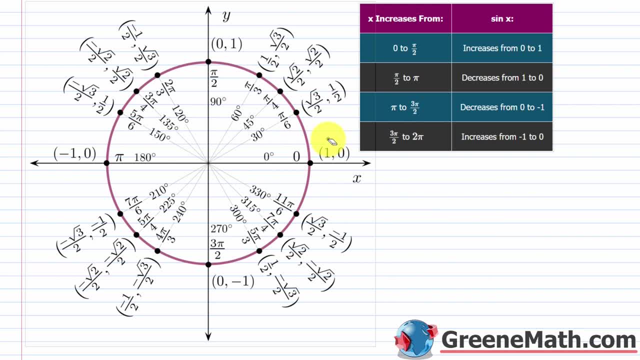 let's go through And let's think about some of the basic point that you're going to get from a sine graph. Okay, So we're going to be looking at: Y equals the sine of X. This is a function, So you can use function. 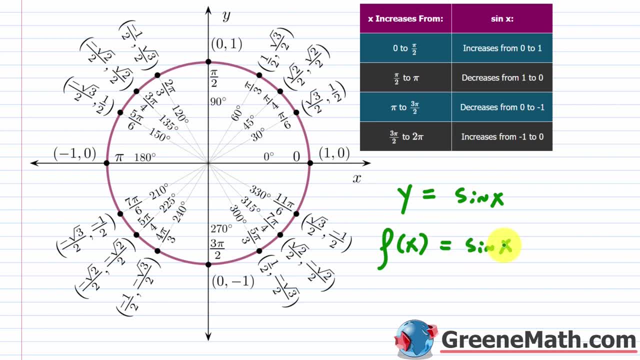 notation: F of X equals sine of X. It's not a one-to-one function, but we'll talk about that later on in the course. Okay, So if we look at these Y values here, we're going to be focused here, here, here, here and here right. So, as we start from an angle measure, 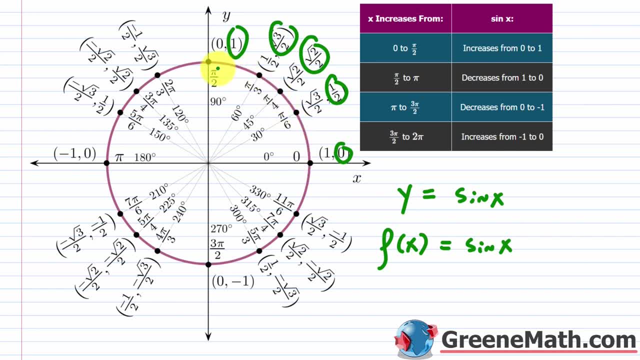 okay, and we go to pi over six, pi over four, pi over three, to pi over two, you'll see that the sine of X or the Y value- okay- is going to increase from zero to a half square root of two over two, square root of three over two to one. Okay, Then, as we go from pi over 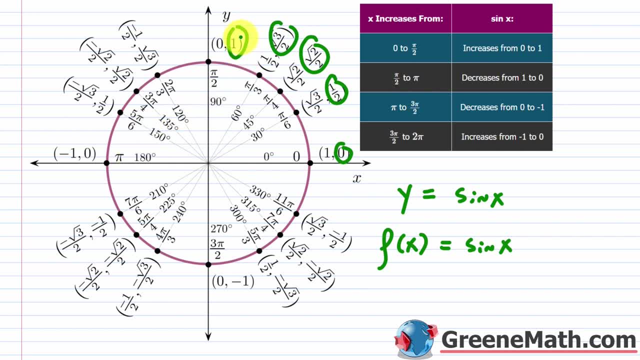 two to pi. this guy's going to now decrease from one down to zero. Okay, So you're going to go to square root of three over two, again square root of two over two, and then one half, and then back to zero. Okay, Then, as we get into the sine of X, we're going to be focusing on the sine of Y. 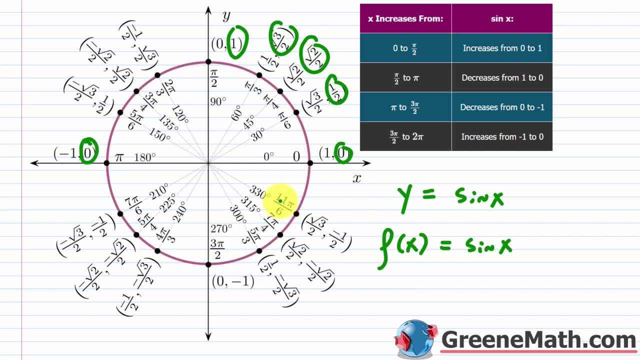 So as we get into our quadrant three and our quadrant four, remember sine is going to be negative. So from pi down to three, pi over two, we're going to be decreasing from zero down to negative one. Okay, So you can go to negative, a half negative square root of two over two and 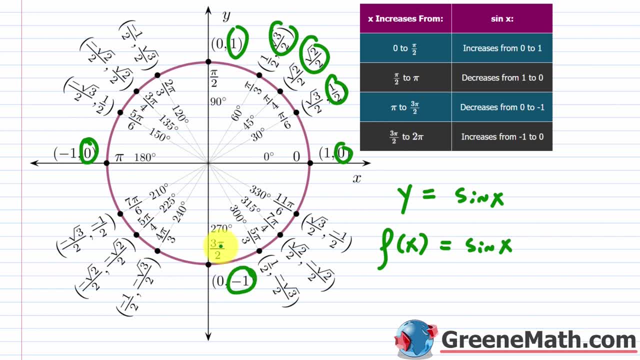 negative square root of three over two. Finally, you get to negative one And then, lastly, from three pi over two, up to two pi, So up to one full rotation. we're going to increase from this negative one back to this zero, right? So you go in negative square root of three over two. 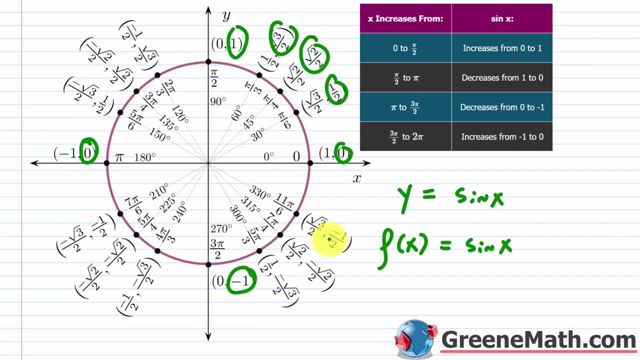 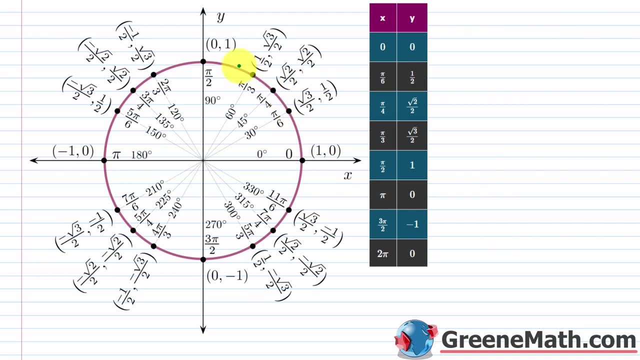 negative square root of two over two and then finally negative one half. Now you do not need all of these values as ordered pairs. You can just start off by taking the first few guys that you get in the first quadrant, along with your quadrantal angles. Okay, And that's basically enough to get started. 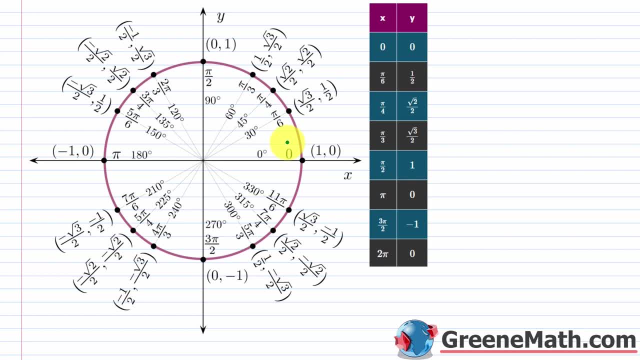 After that I'll show you that you really only need five key X values to draw this guy over one period. You're going to draw a wave like function. Okay. So if we start with zero, that's our angle measure- The Y value is zero, Then pi over six, you get a half. 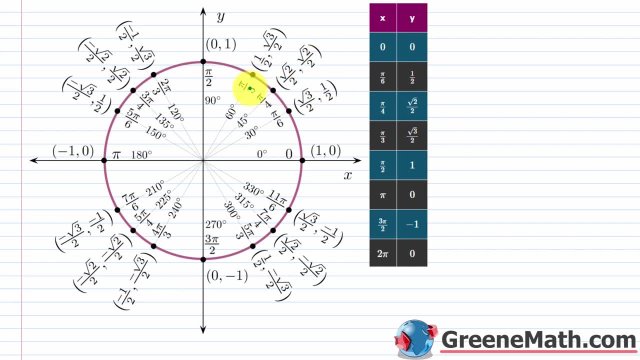 then if we do pi over four, you get square root of two over two. Then if you do pi over three, you're going to get square root of three over two. Then if you do pi over two, you get one pi, you get zero. three pi over two, you get negative one and two pi, which is one full. 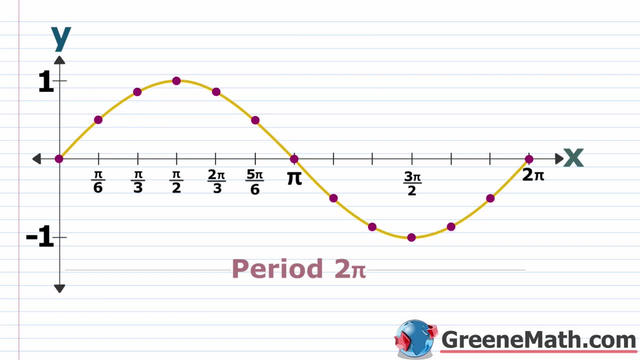 rotation. You are back to zero. All right, So now that we have some basic points, let's go through and draw our first graph of. I'm going to go ahead and label this as F of X is equal to the sine of X. I'm specifically going to say here because this is over one period, So 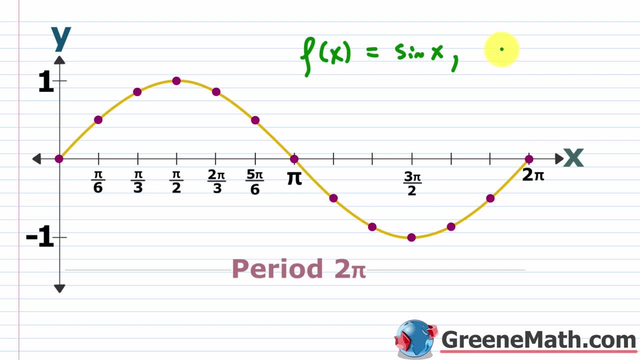 from zero to two pi, So one rotation. I'm going to say that X is greater than or equal to zero and less than or equal to two pi. I'll show you in a minute that this continues to the right and to the left forever. Okay, So what we've done here? we've put a little bit of detail into this. 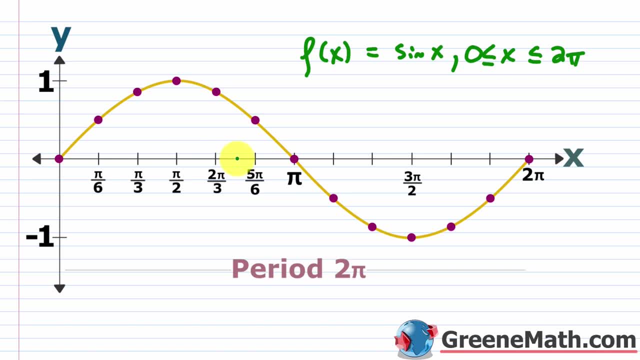 more detail than you really need. You'll see. I have these notches that are going to be in increments of pi over six. We're going to start out with an angle measure of zero. Okay, Again, the sine of zero is zero. So your X value is zero, Your Y value is zero. Okay, Then, as you get, 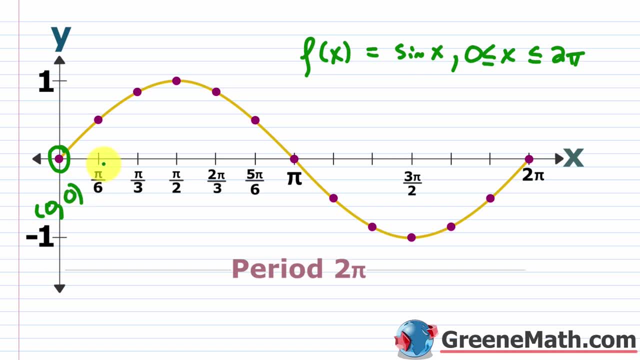 to pi over six. what's going to happen is your sine of pi over six is a half. So you can say this: right, here is a half. Okay, You can label that: this is pi over six, comma one half, And I'm trying to make that a little bit better here. Okay, Then, as you continue, then you have your. 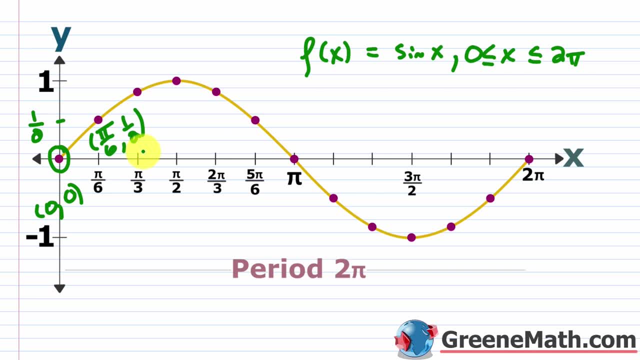 pi over three and the sine value for that is going to be square three over two. So this right here would be your pi over three, And then square root of three over two. Okay, And then at pi over two, you get to the maximum. 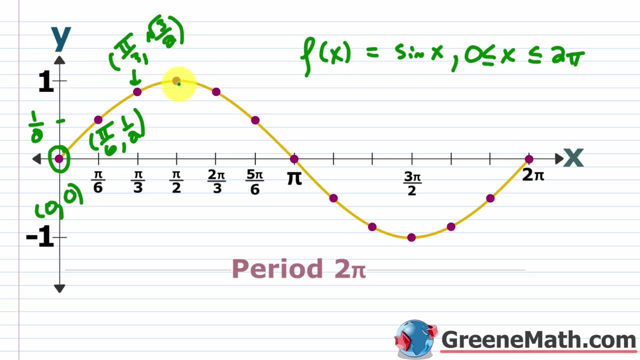 Y value, which is one. Okay, So that's right there. Then you start decreasing again. Remember, after pi over two you're coming back down to a Y value of zero. So you're decreasing. So now this is your maximum. Then you're going to come back to your square root of three over. 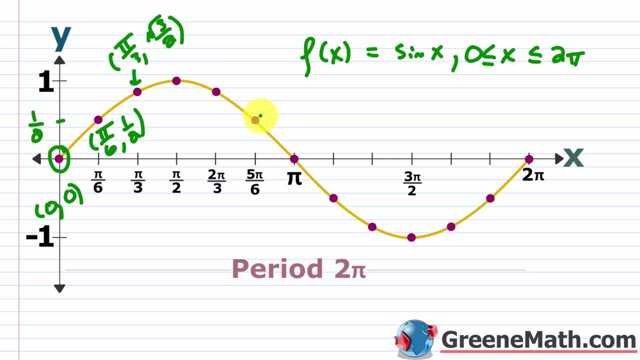 two in terms of your Y value. You're going to come back to your one half in terms of your Y value, And then you come back to zero or an X intercept when you get pi. Okay, So then, as we continue from pi to three, pi over two, we are decreasing from zero down to negative one. 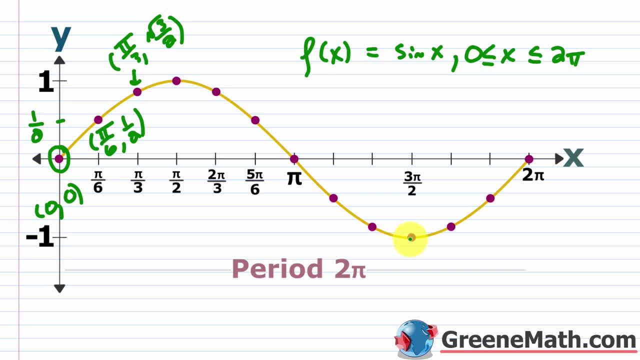 which is the minimum. Okay For the Y value. Then, as we go from three pi over two, back to two pi, back to one full rotation, we're going back to zero. This just goes directly in line with what we're doing on the unit circle. Now, when you graph these guys, let me erase all of this. 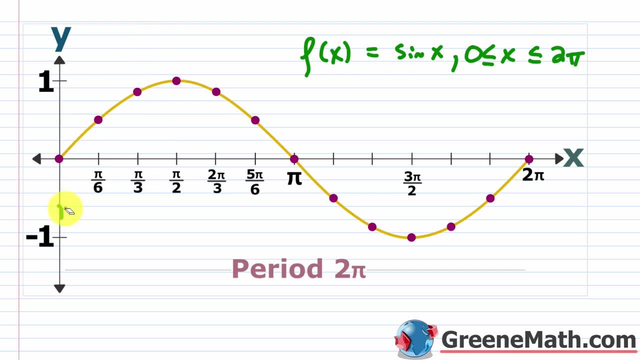 You really do not need all of this detail. Okay, I put some notches here in terms of pi over six. Typically, if you're asked to graph these guys, you're going to have to do that. So if you're over one period, you're going to make five notches for the five key X values. Okay, You're. 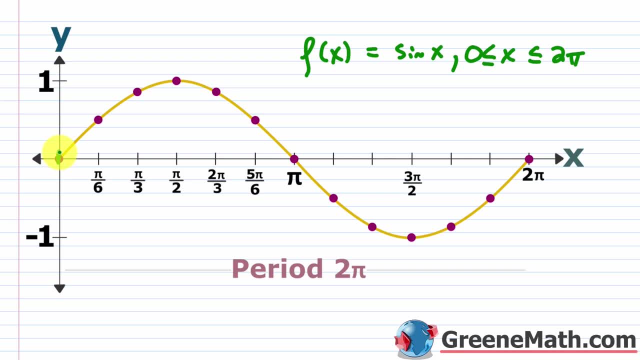 going to have a starting point, You're going to have a quarter point. Let me mark these off So you have a starting point, a quarter way point, a middle point, a three quarter way point and then an ending point. Okay, For the basic sign graph. it's really easy because these key X values. 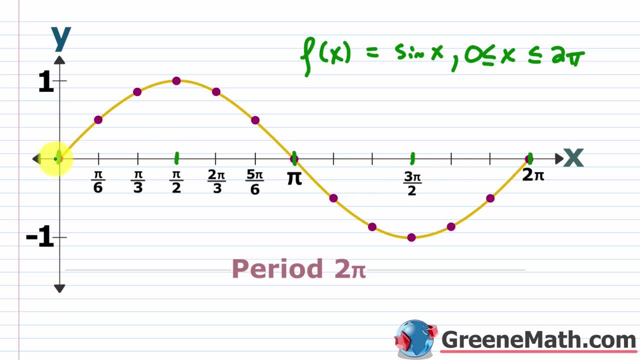 are going to be your quadrantal angles, right? So this is, if you think about it in degrees, if that's easy to remember, this is zero degrees, 90 degrees, 180 degrees, 270 degrees and then 360 degrees. Okay, So very easy to get those five values. 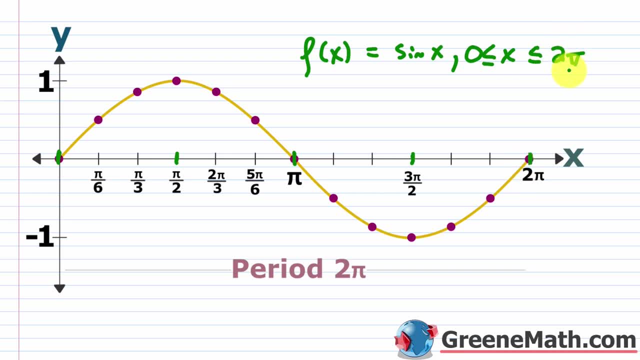 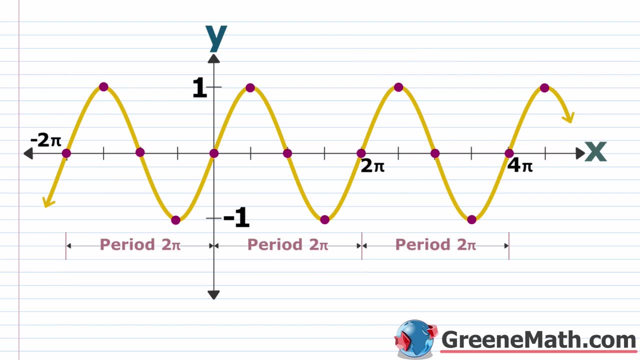 I'm going to talk about in a moment splitting up the period into fourths, but I'll get to that in a moment. So let's go down here and I want to think about what happens when we extend this to the right and to the left. Well, again, if I start off here with my next value of zero, let me write: 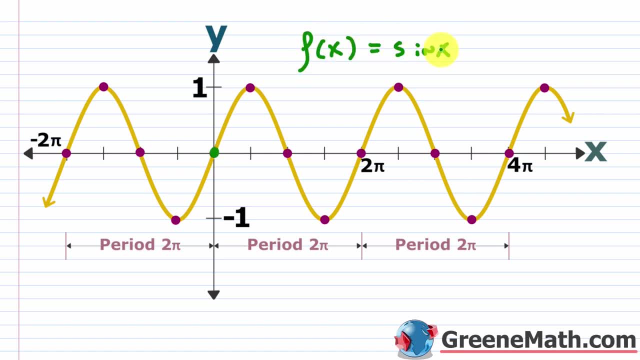 this out. So now this is: F of X equals sign of X. Okay, No restriction, We're going all the way through One full rotation, or one cycle would be. I would go up to one. I would go back through my X. 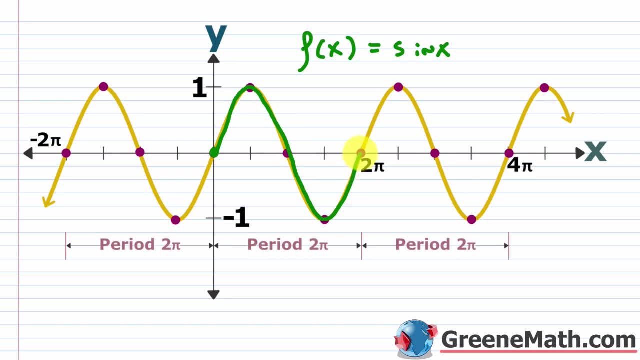 intercept down to the minimum and then back up to my X intercept. Okay, So this is one cycle, or one rotation on the unit circle. Every other part of that graph is just made up of repetitions of this. Okay, You can see this is called a sine wave. Okay, So when you graph this guy, you're going. 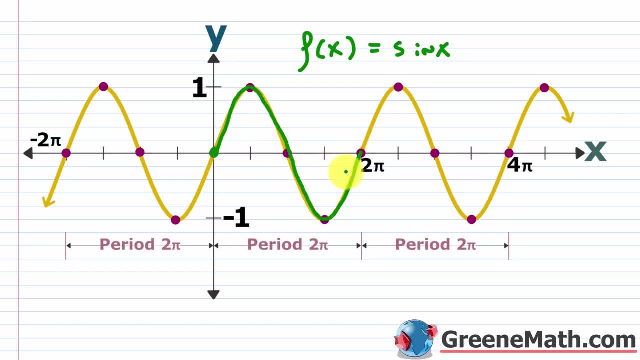 to have your five key points, So one, two, three, four, five, Given by the five X values which I'll talk about in a moment, And then the corresponding Y values, obviously, And then you're going to sketch that wave and just continue that wave indefinitely to. 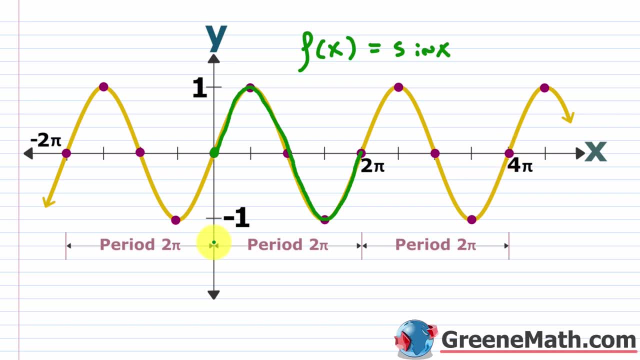 the right and to the left, based on what your teacher says. Okay, You've seen that. I've marked this off in increments of two pi, So that's your period. And another way we want to think about this. if you're going this way, okay, Think about what a negative angle measure means. 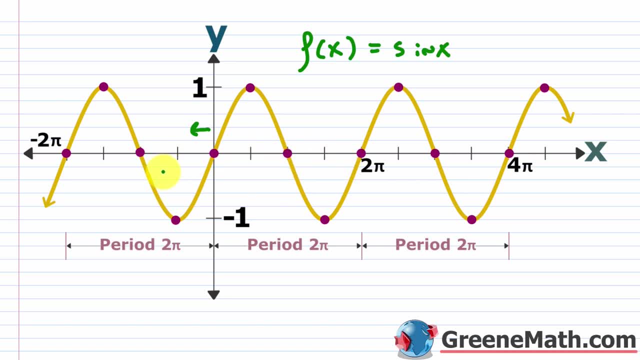 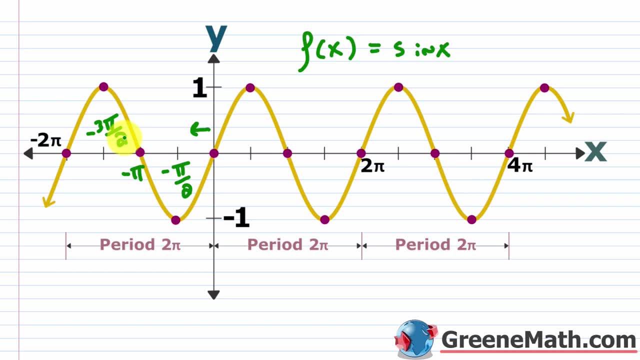 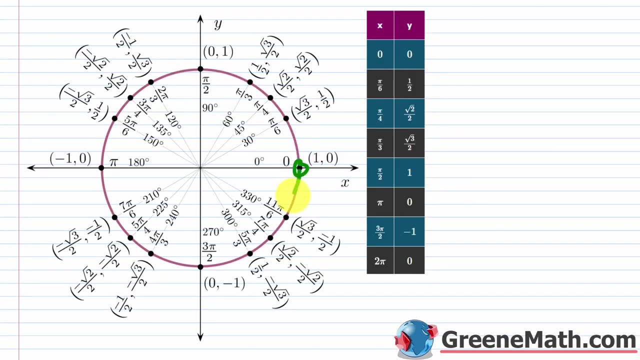 Remember what it means to have a negative angle. It means I'm rotating clockwise. If I go back to the unit circle, if I start here and I rotate this way, okay, I'm going to end up with negative pi over two, which is coterminal with three pi over two. So the sine value is negative one. Then, as I 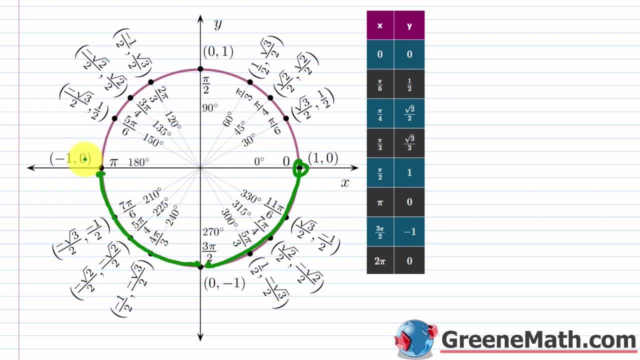 keep going, I'm going to end up with a negative pi. The sine value is zero, right? This is coterminal with pi. Then, as I go and I continue, then I'm going to end up with negative three pi over two. 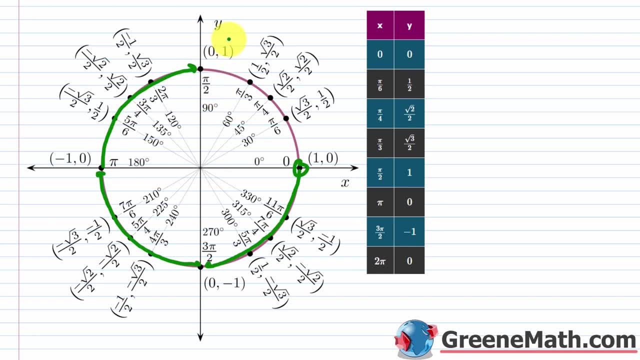 This is coterminal with pi over two, So the sine value here is going to be one. And then finally, as I make my full rotation going clockwise, now, okay, I'm going to end up with negative two pi And my sine value there is going to be zero once again. So when you return, 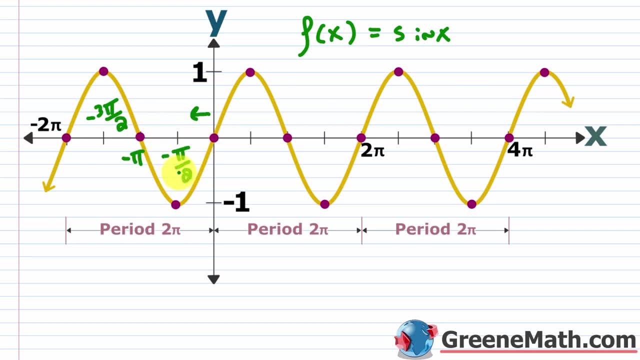 if you think about this again, as we get to an x value of negative pi over two, our y value is going to be negative one. As we get to an x value of negative pi, our y value is going to be zero. As we get to an x value of negative three pi over two, our y value is going. 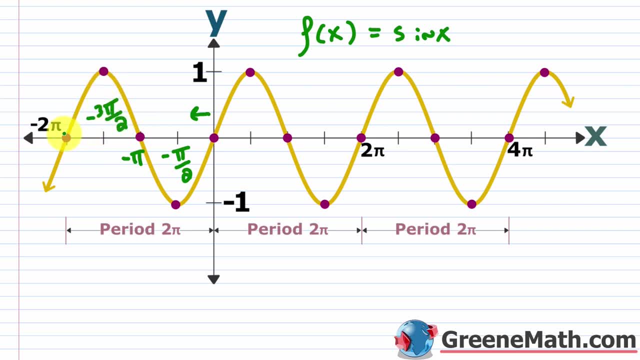 to be one As we get to an x value of negative three pi over two. our y value is going to be one As we get to an x value of negative two pi, our full rotation we're right back to zero. We're. 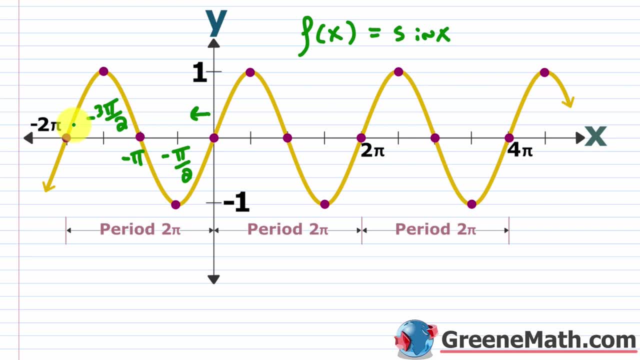 hitting the x intercept. Now here are a few things that you absolutely need to know when you work with the sine function. First off, this guy is continuous across its entire domain. The domain is a set of real numbers. okay, So that means you can plug in any real number you want. 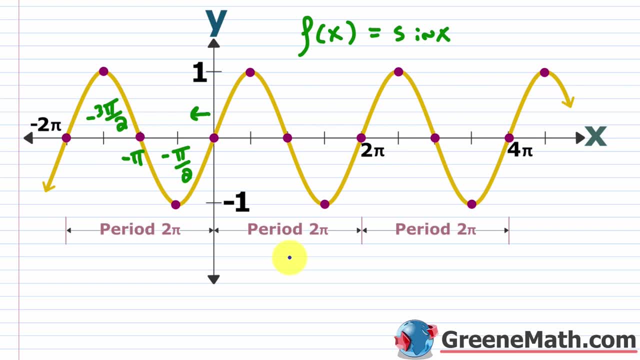 and you'll get a corresponding y value. It also means that when I say continuous, you can graph this guy without ever lifting your pencil. There's no holes, no gaps, nothing like that. Okay, Additionally, when we think about the x intercepts, so you think about here and here and 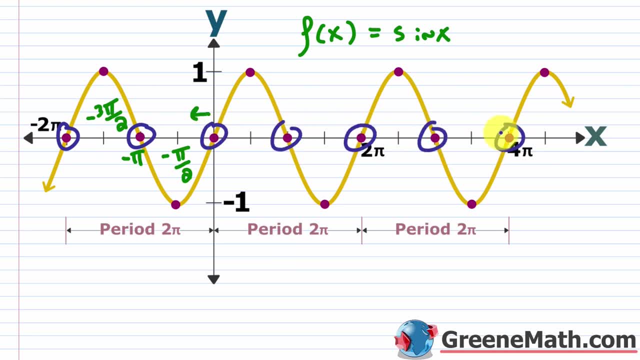 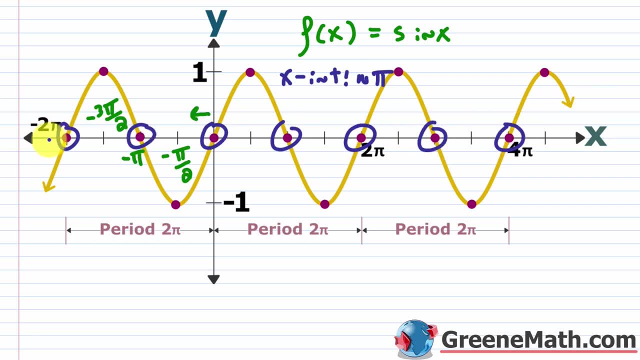 then four pi Work going negative, so you'd have basically negative pi and negative two pi, so on and so forth. Now your range for sine and also for cosine is from negative one to positive one, So the minimum y value would be. 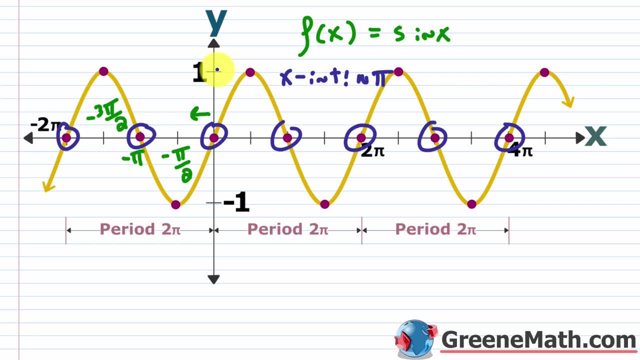 negative one, and that's included. and the maximum y value is positive one, and that's included. So we can say our range- and let me put the e there, forgot that- So our range is going to be from negative one to positive one, like that. Now, the last thing I want to talk about is that. 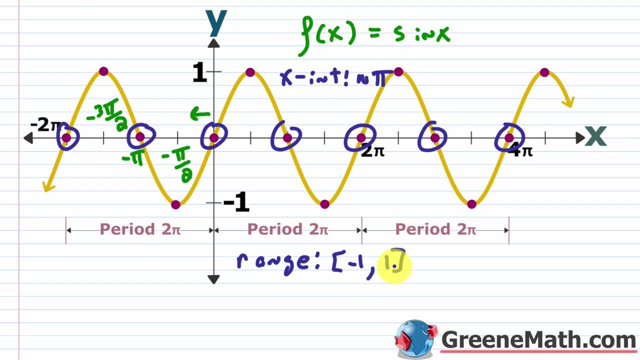 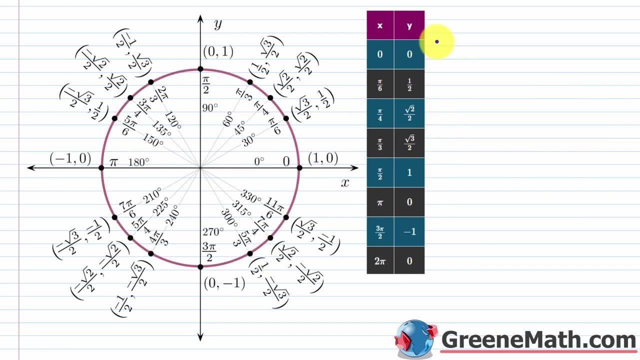 this graph is symmetric with respect to the origin. So when this happens, we call this an odd function. So let me go back to the unit circle and let me demonstrate this real quick. For an odd function, f of negative x is equal to: 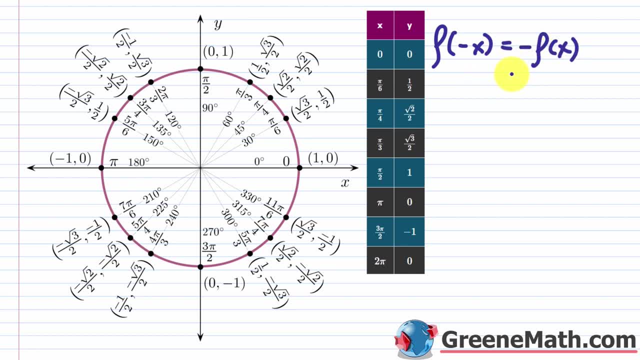 the negative of f, of x. Now, this is going to come up in our section on identities. We're going to need this, what we call negative angle identity, to rewrite things, But for right now, I just want you to understand this concept. If I have the sine of negative x, let me put this in parentheses. 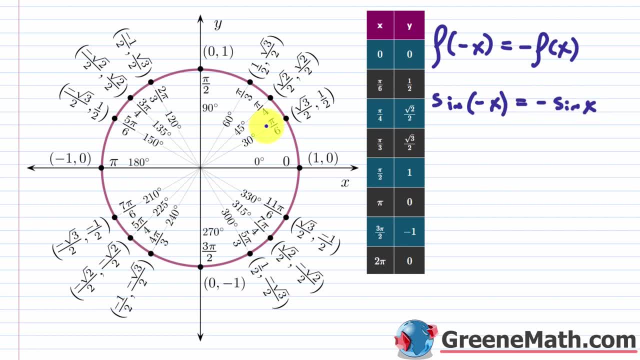 this is equal to the negative of the sine of x. okay, Let's just go back to this. pi over six. If I do the sine of, let's say, negative pi, what would that be? Well, that would be me starting here and rotating clockwise. 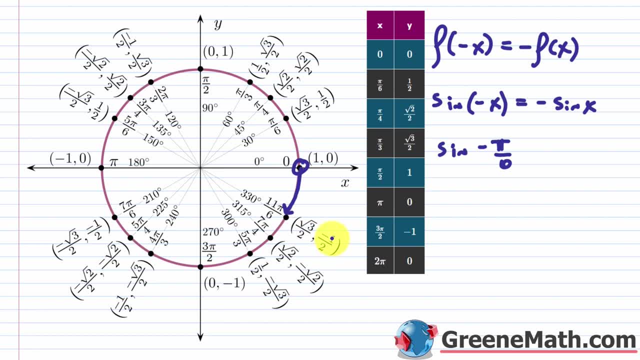 okay, to right there. It's coterminal with 11 pi over six, So the y value for that point would be negative one half. So this is negative one half. Let me write that This is equal to the negative of the sine of x. okay, I have a negative x, I want just x. So the negative of the sine of 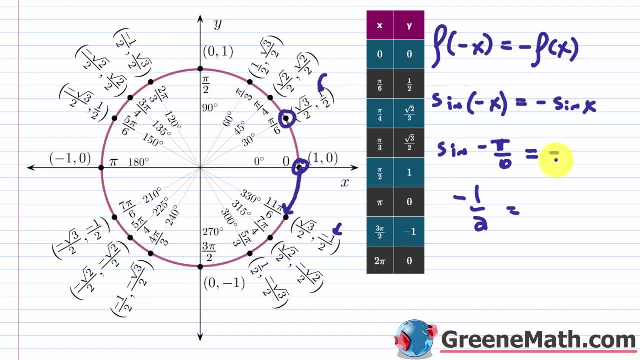 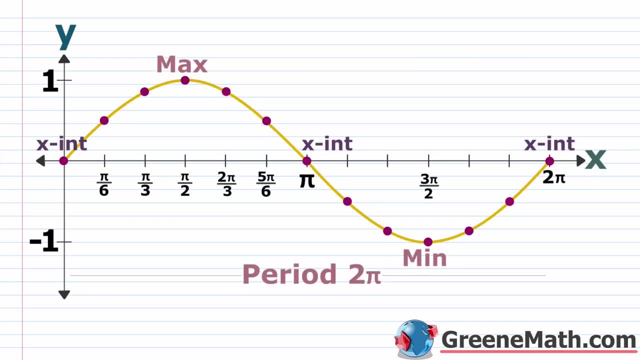 pi over six. So the sine of pi over six is given by this y value here. So this is going to be the negative of sine of pi over six, which is going to be negative one half. So this is going to be negative one half as well. Okay, let's move on now and talk about graphing variations of the 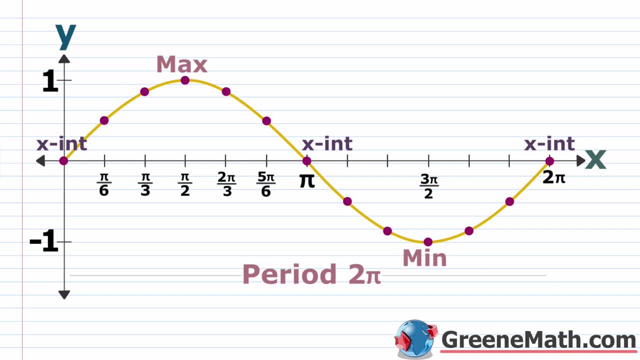 sine graph. I'm going to go through all the different transformations that you're going to come across. We're going to start off with a vertical stretch or vertical compression, okay, And in order to graph these variations by hand, what you want to have are the x-intercepts. 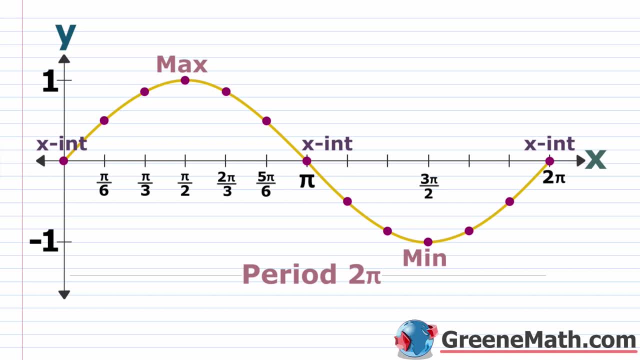 You want to have your maximum point and then your minimum point. okay, if you're looking at one period. okay. So when we look at one period or one cycle, you think about your x-intercepts or your basic sine graph. You want to have your x-intercepts or your basic sine graph. 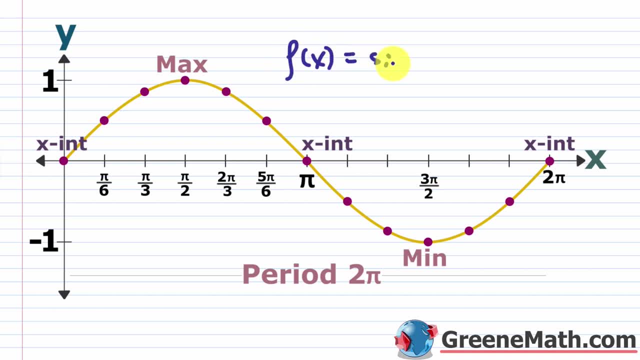 Let me write this out again. So f of x is equal to the sine of x, or x is greater than or equal to zero and less than or equal to two pi. Your x-intercepts occur at the beginning, the middle and the end of your period. okay, So zero pi, two pi. okay, Then, in terms of your maximum, and 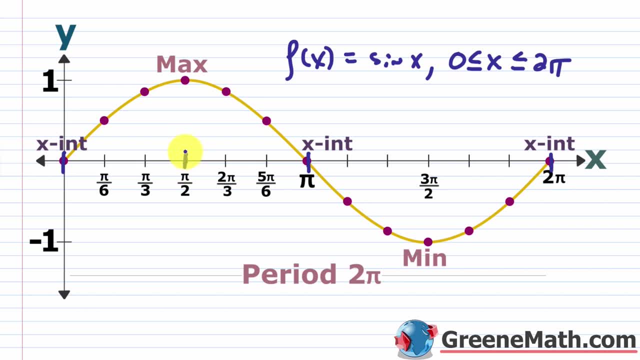 your minimum. your maximum is going to occur at a quarter way through the period. okay, So two pi divided by four, two pi times a fourth, that's going to give you pi over two. And then your minimum is going to occur at three quarters way through your period, So three. 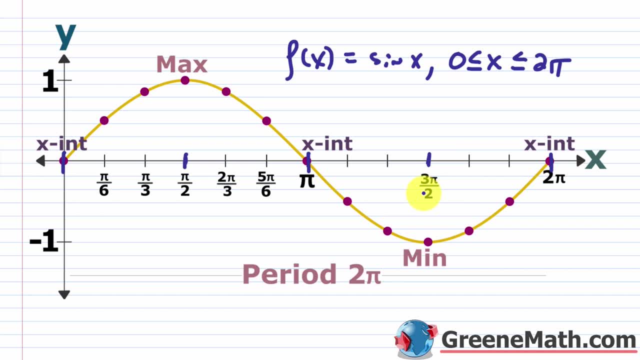 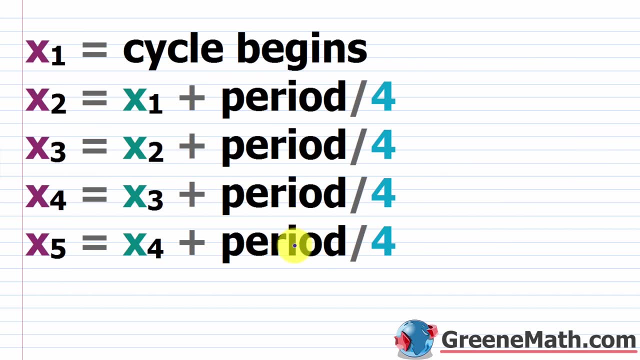 fourths times two pi, we give you your three pi over two, okay. So what you want to do to get these x values in any situation is you want to set yourself up a little table? okay, Or you could say just some scratch work, And you want to first divide your period by four? okay. So with the 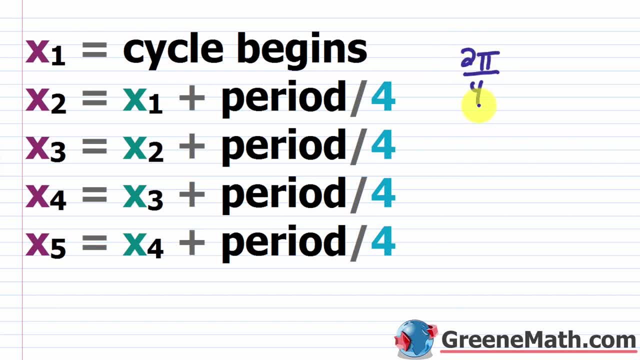 basic sine function. the period is two pi. okay, We're going to divide this by four. So we cancel this with this and get a two. So basically, you have your x-intercepts. you're going to have your pi over two, okay, So you're going to start off where your cycle begins For the basic sine. 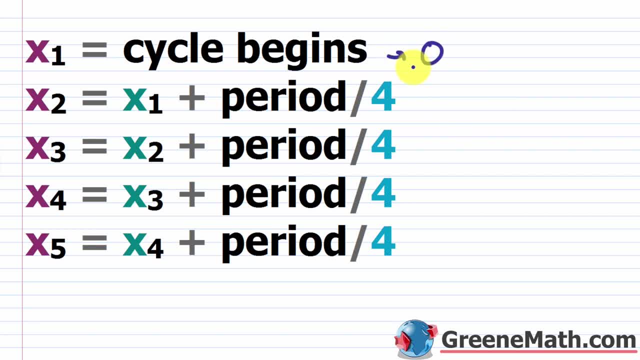 function, it's going to start at zero. okay, So let me put zero here. And then what you're going to do is you're going to just keep adding pi over two to the previous value. So here x sub two, or the second x value is this x sub one, which is zero, plus your pi over two, So that's pi over. 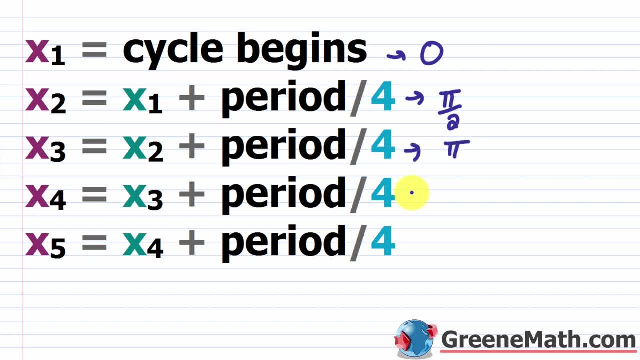 two, okay, And then here it's pi over two plus pi over two, which is pi, and then plus pi over two again, which is going to be three pi over two, and then plus pi over two again, which is going to. 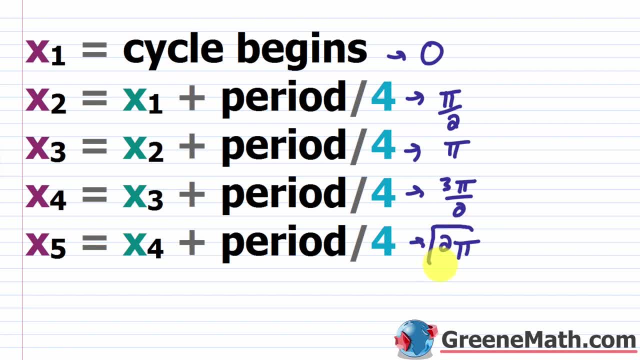 Typically as a check, a lot of books will say: take your ending value minus your beginning value, so two pi minus zero. If that equals your period, you're pretty much good to go. okay, Now, that doesn't mean you didn't make some mistake in between, but at least you know that your cycle 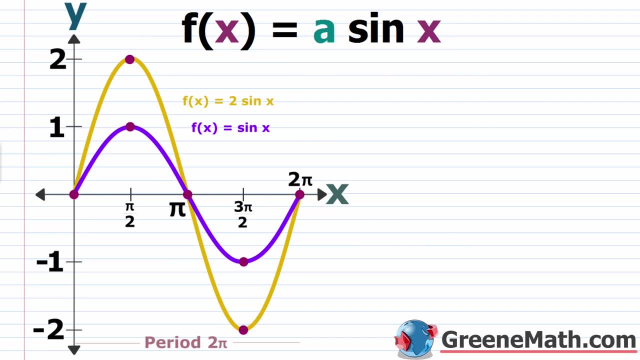 is the right length, All right. so let's start talking about some of the function transformations that we're going to see. The first type is very, very easy. This is where we have a vertical stretch or a vertical compression. You'll recall from earlier in the course if we have something. 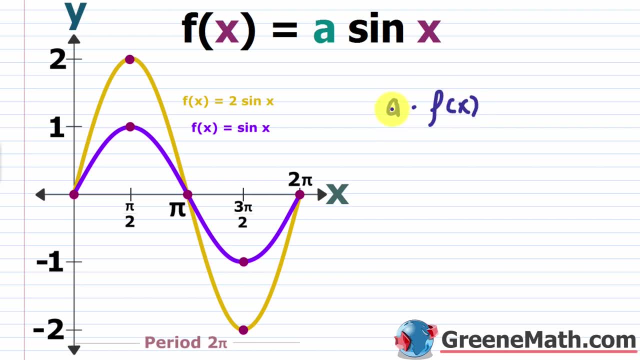 like a multiplied by f of x, we're going to have a vertical stretch and we're going to have a f of x. Basically, if this a value, we'll say the absolute value of that. if that's greater than one, you're going to have a vertical stretch If you have the absolute value of a being greater. 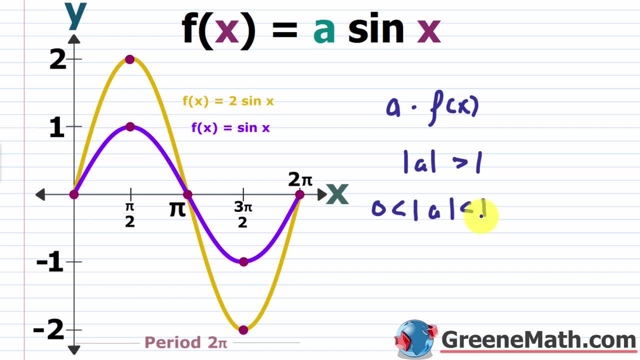 than zero and less than one. now you're going to have a vertical compression, okay. So all your function values, or your y values, are being multiplied by this guy a here. okay, So what we see here is we have f of x is equal to a. that's multiplying the sine of x. So the original 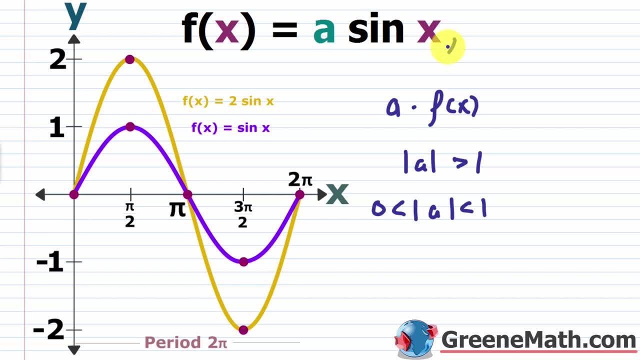 function is sine of x. a is now multiplying that, and I'm specifically going to say that a is any real number that is not zero, okay, So some non-zero real number. So the example we start with is f of x equals two times the sine of x. So basically we know that, since 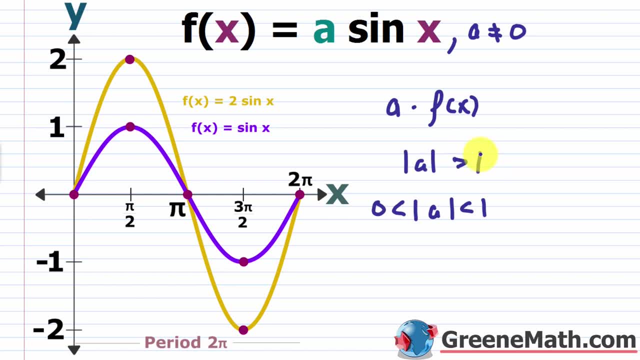 this is a two and the absolute value of two is two and that's greater than one. this would be a vertical stretch right, Because all the function values, all the y values, are being multiplied by two. when we compare it to the original function, f of x equals sine of x, And you can see this So. 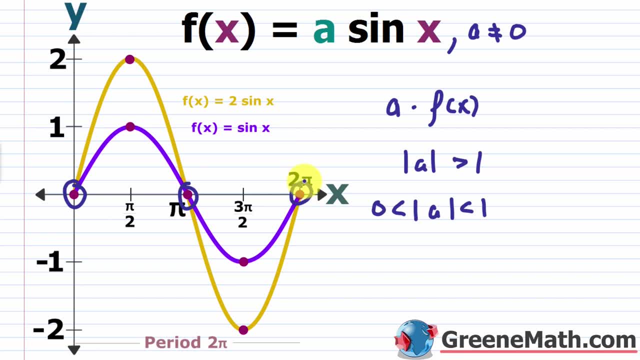 that's here, here and here. Obviously, the y values are zero, so those are going to stay the same, because zero times two is still zero. But if you look at this maximum y value of one, okay, if you multiply that by two, you're now at two. okay, One times two is two. If you look at the 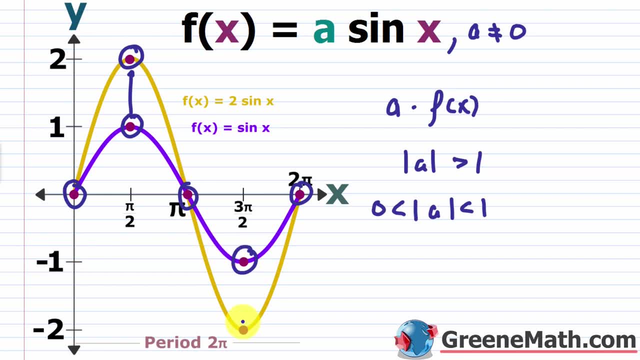 minimum y value, which is negative one. you multiply that by two, you're down here to negative two. okay, So this guy has been vertically stretched by a factor of two. Now, when we think of this form, it's still going to be two pi. okay, So we haven't introduced any type of shift. 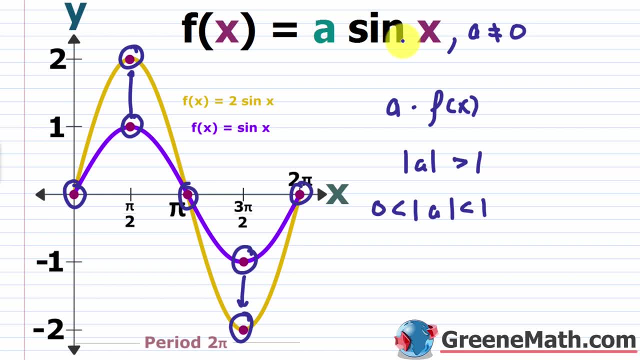 We haven't introduced any type of horizontal stretch or compression, So the period is still two pi. We're still starting out with an x value of zero, So you still have the same five key x values at zero: pi over two pi, three pi over two and two pi okay. So basically to get these. 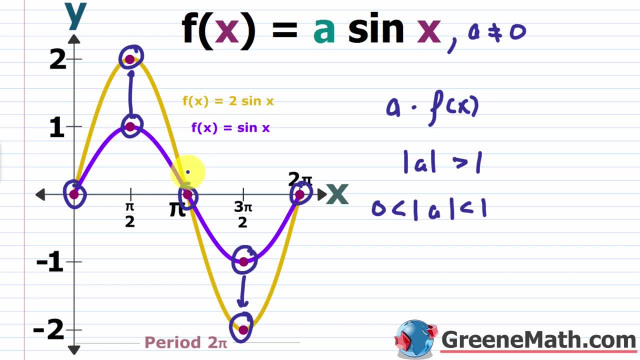 points. you really just need to think about the fact that you're multiplying the y values from two. okay, That's all you really need to do Now. I'm going to talk about in a moment the fact that you can use this a value to find your maximum and minimum y value, but we're going to talk about that. 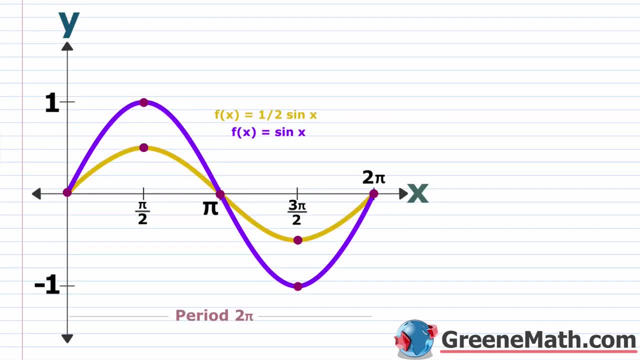 later on when we talk about the amplitude. Okay, let's look at another example. Again, I'm working with. f of x is equal to a times the sine of x. Here we have f of x equals one half times the sine of x. So what do you think is going to happen here? We're going to have a vertical. 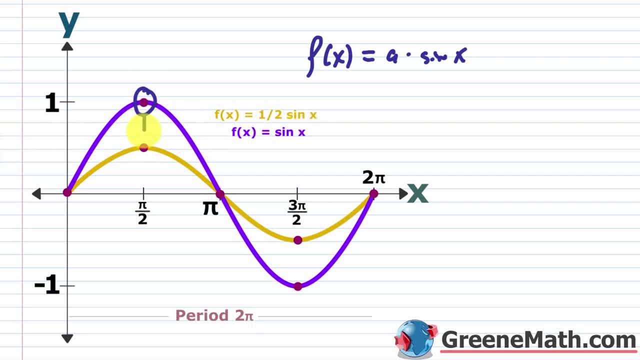 compression. okay. So basically all your y values now are multiplied by the sine of x, So you're by a half and that's compressing your graph. okay. So again you get your x values in the same way. The period has not changed, So it's still going to be zero pi over two pi, three pi over. 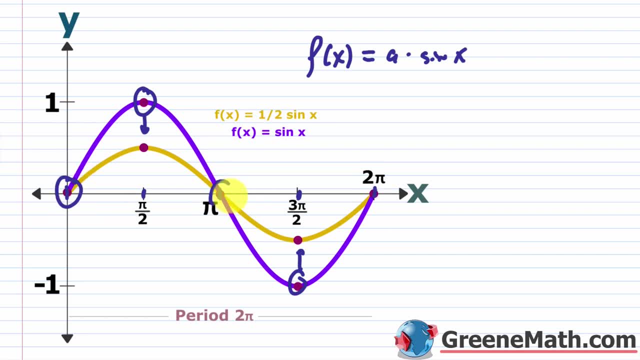 two and two pi. That part's really easy. So the x intercepts, the y values, are always going to be zero. And then for these y values here on your new graph again, you can just multiply the previous ones by a half, or you can evaluate the function there, Or again, I'll talk in a moment about how. 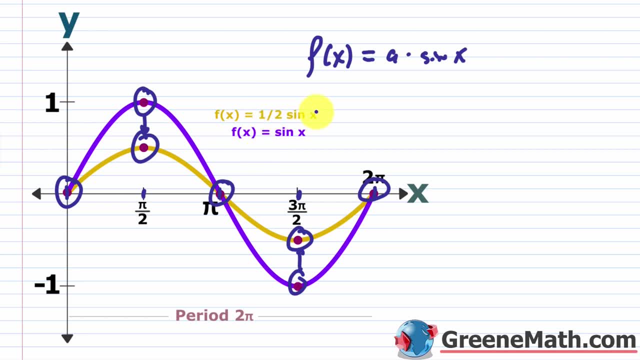 to get the minimum and maximum value. You might notice that when we had two times the sine of x, it was two and negative two. When we just had sine of x, it was one and negative one. Here we have one half times the sine of x and it's basically a half I can put. 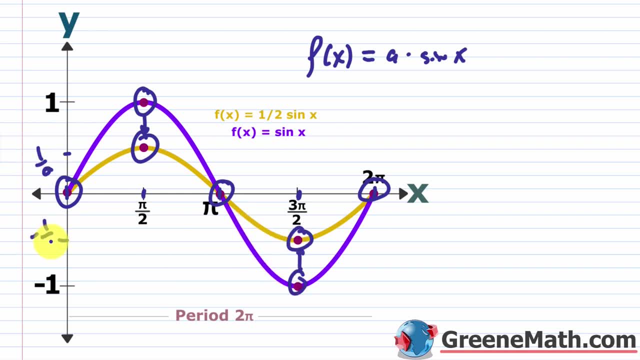 that in This is a half, And then down here this is negative one half. So you see, the pattern is that your maximum and minimum is related to this right here. We'll talk more about that in a moment. All right, let's take a look at one more of these in this form. So now we're going to look at f of. 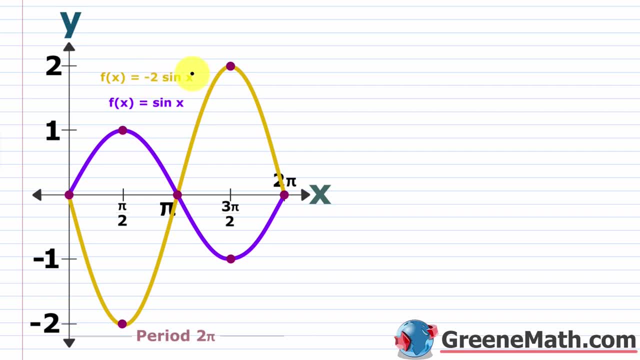 x equals negative two times the sine of x. So you actually have two different things going on. One, you have a vertical stretch of a factor of two And then you have that negative there that's going to cause a reflection across the x axis. So, compared with the graph of f of x equals: 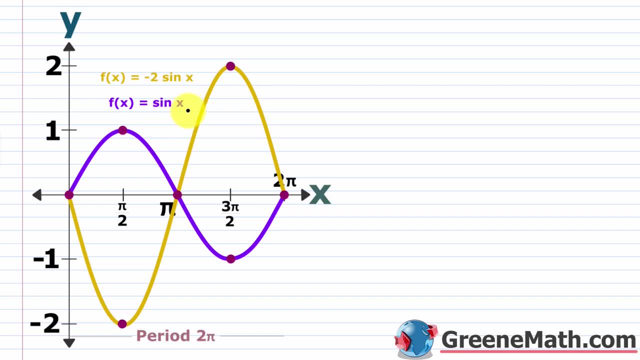 the sine of x. basically all your y values are multiplied by negative two. So again you have the same period, so you have the same x intercepts. So you're going to have this guy, this guy and this guy. Those are going to be the same. Y values are still going to be zero. But when you 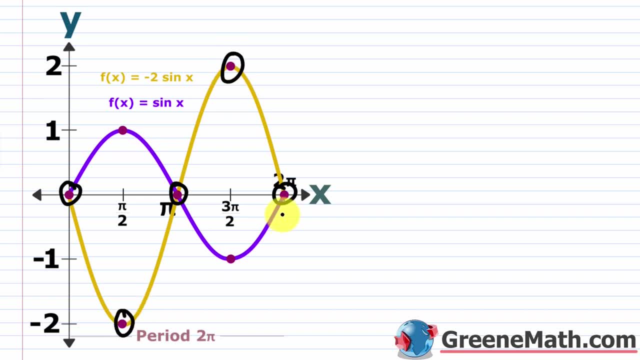 look at this guy and this guy. okay, you can go from your basic sine graph and you can just multiply those y values by negative two. So one multiplied by negative two gives you this negative two, And then negative one multiplied by negative two is going to give you this positive two. Okay, 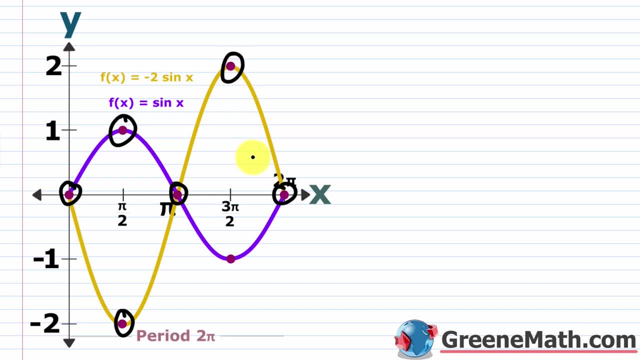 And if you think about this in terms of your f of x equals two times the sine of x. again the negative there. if you have the negative of f of x, whatever you're working with, it's a reflection across the x axis. So if we go back, 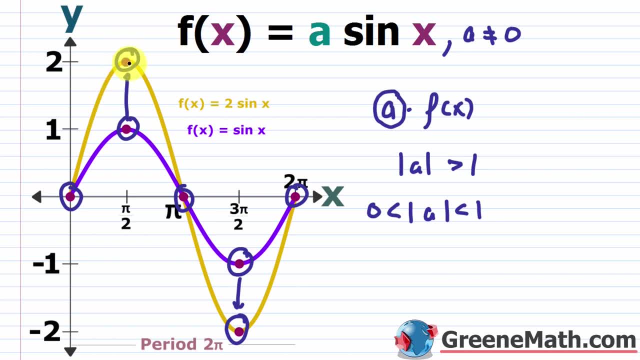 and look at this guy one more time, you can see that we have this peak here, okay, where your x value is pi over two and your y value is two. Okay, So this is going to be reflected across the x axis, And so now this is going to be your minimum point, right? So at pi over two. 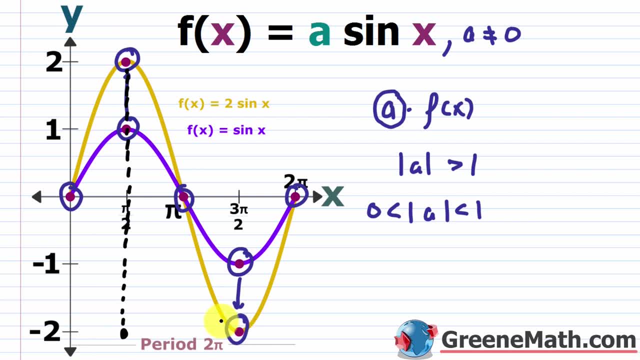 comma negative two, And this guy right here which was your minimum right, where you had three pi over two comma negative two. Well, now this is going to come up and be your maximum. it's getting reflected across the x axis, So now it will be three pi over two comma positive two. 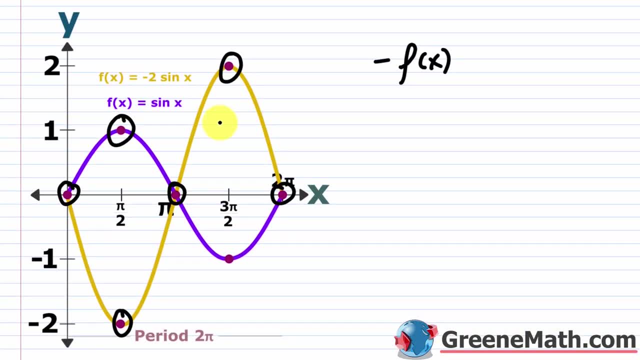 If we go back, you'll see that's exactly what we have here. Okay, so let's make a few generalizations. You should notice that this is negative two here, and the maximum is still two, and the minimum is still negative two. So what I would say here is that if you have this f of x, 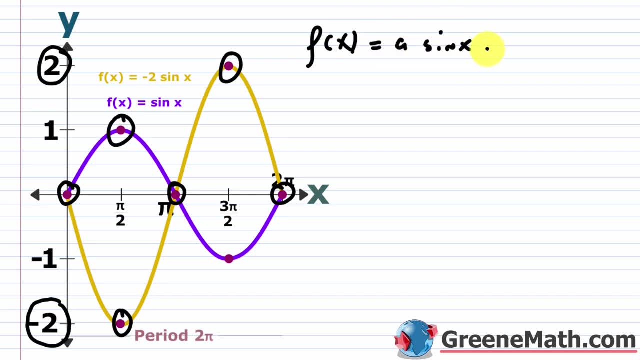 is equal to a times the sine of x, where again we're going to say: a is not zero, but it could be any real number you want other than that. Then, basically, if you think about the range, okay, and this is going to give us our maximum y and our minimum y. 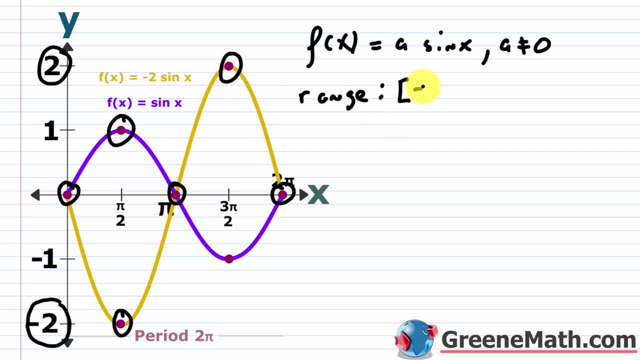 then what I do? I'll put some brackets here and I'll say it's from the negative of the absolute value of a to the absolute value of a, And I'm using these square brackets here because these values are included, right, If we look at this negative two here: the absolute value. 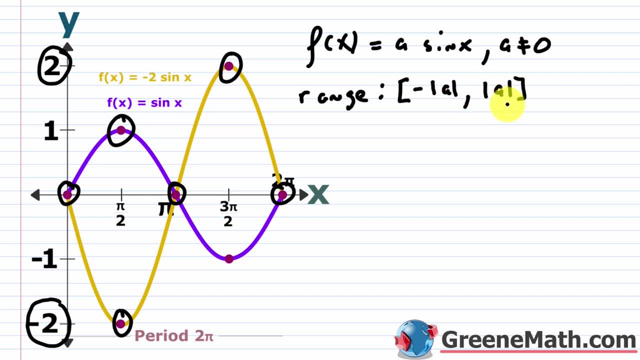 of that is two. So you'd want negative two to positive two. Again, both are included. If you went back to a half, it would be negative a half to positive a half- both are included. If you had positive two again, it would be negative two to positive two- both are included. 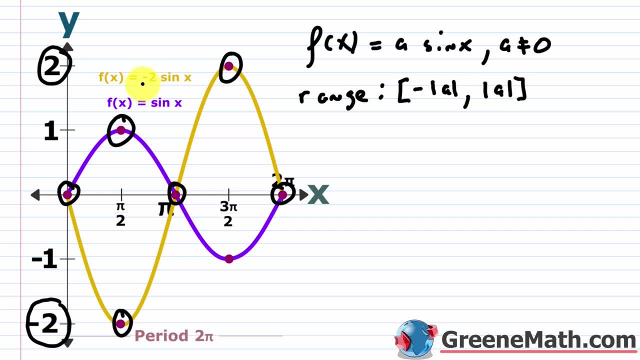 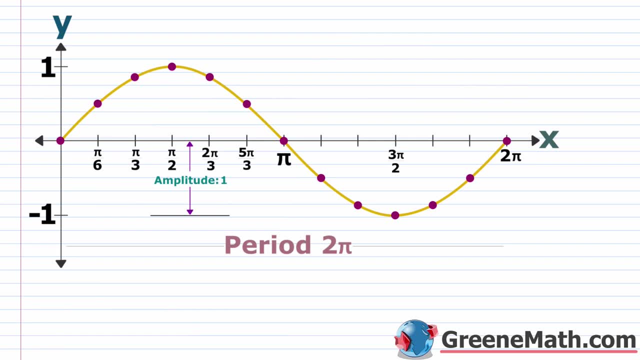 If this was 57, then it would be negative 57 to positive 57, you know, so on and so forth. All right, The next concept I want to talk about is known as the amplitude. This is something you need to know. 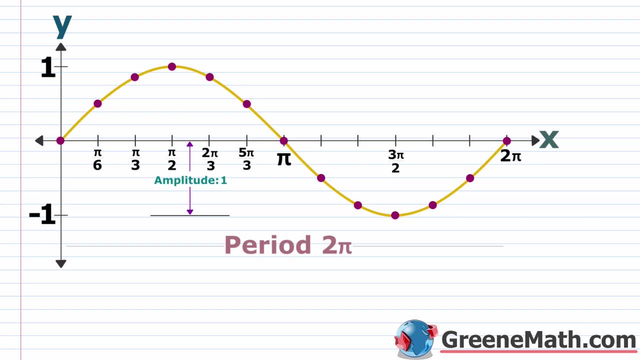 when you work with the sine or cosine function, And it's going to be the same for the basic sine graph and also the cosine graph, which we'll talk about later on. So over one period, let me write this out. So f of x equals the sine of x. Again, x is greater than or equal to zero and less than. 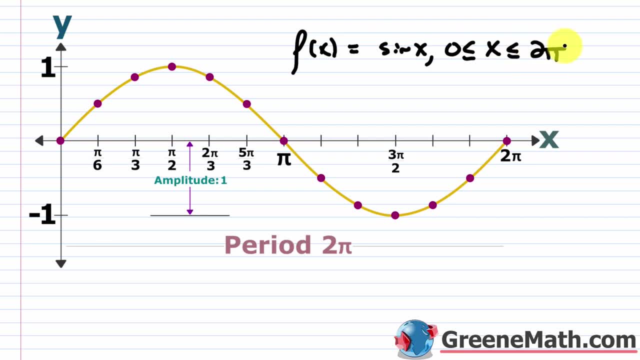 or equal to two pi. So we're looking at this right now And basically, you'll see that I've written: the amplitude is one. So what does that mean And where does it come from? Well, basically, when you think about the amplitude, you're thinking about something that describes the height. 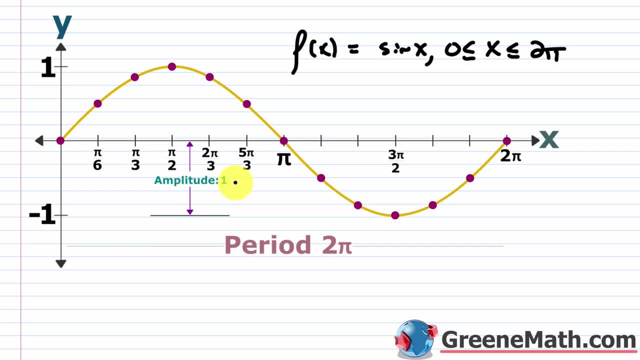 of the graph, both above and below your horizontal line that passes through the middle of the graph. So for the basic sine or cosine function, that's going to be your x axis. okay, that's going to be your x axis. So it'd be the line: y equals zero. Okay, So from this guy, right. 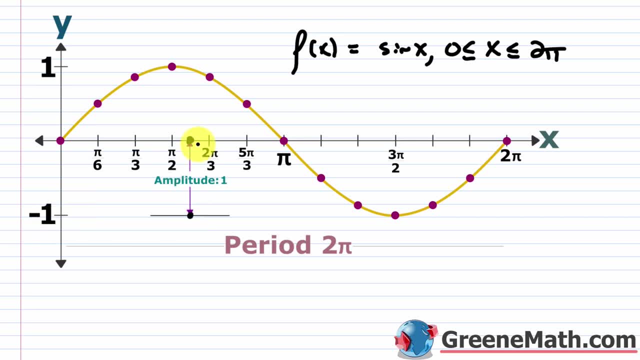 here, to this guy right here: your minimum y value is negative one. It's a distance of one. Or you could say: from right here to up here, that's a distance of one as well. however you want to draw Now, the formula we use is basically to grab the a value. 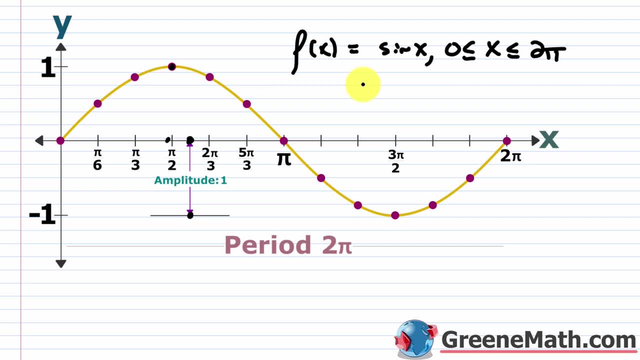 and take the absolute value of that and that's going to be your amplitude. Here you can think about your a value being one. Okay, so the absolute value of one is one, So the amplitude is one. A more precise definition comes from the fact that you're taking half of the difference between the 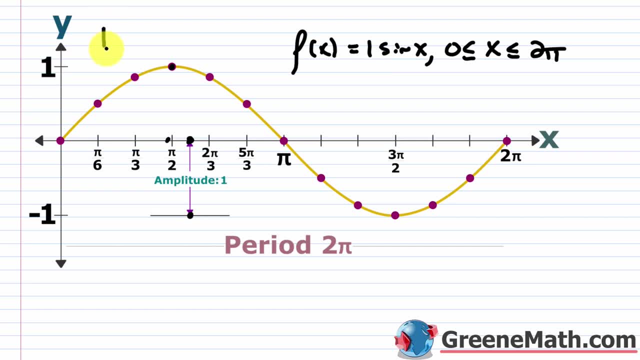 maximum and minimum values. So if you take your maximum and minimum, you're taking half of the maximum, which is 1.. You subtract away your minimum, which is negative, 1.. Minus the negative is plus a positive. So this becomes 1 plus 1, which is 2.. If you took half of that, you're right. 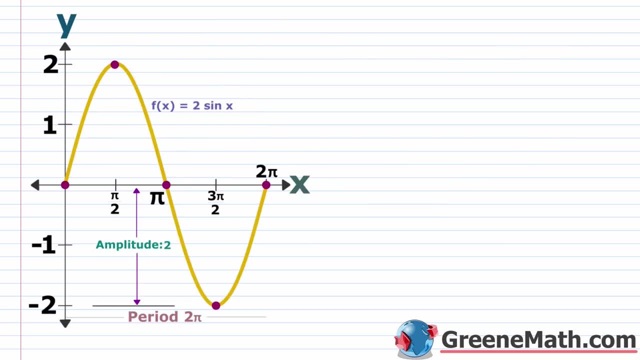 back to 1.. If you want to look at another example of this, again, we've been working with f of x equals 2 times the sine of x. Again, just take this number out in front, which in this case is a 2.. 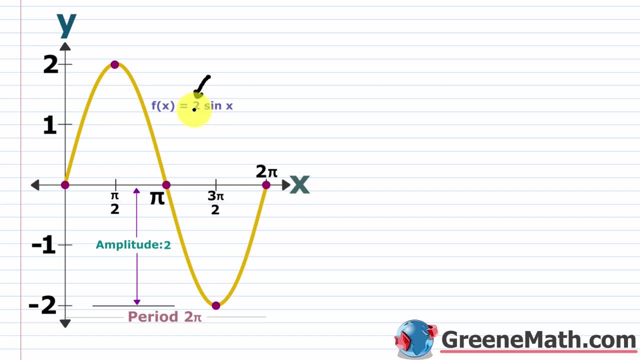 Take the absolute value of it. So if it was 2 or negative 2, the amplitude is just going to be that number And again you can see the distance from this guy right here down to your minimum. That's going to be a distance of 2 units, And again you could just go 2 minus a negative 2.. 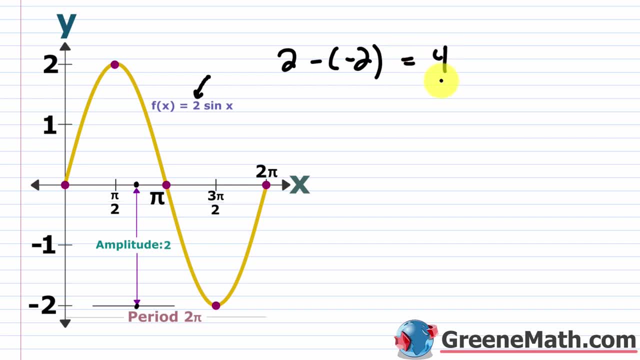 That's going to be positive 4. You half that and you're back to 2.. If you wanted a more generic formula again, you can go: f of x equals a times the sine of x where a is not 0. And you could. 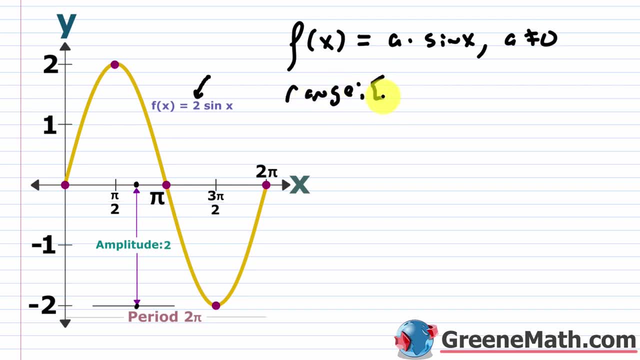 say: OK, well, I know the range. I know the range from earlier is from the negative of the absolute value of a to the absolute value of a. And you can say: OK, well, I know the range from earlier to the absolute value of a. So that tells me that the minimum y value would be the negative. 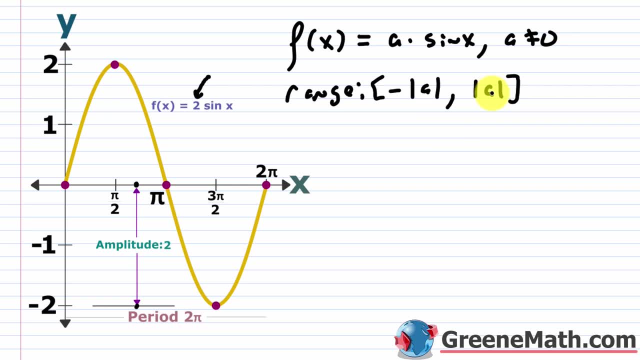 of the absolute value of a. So let's just go ahead and say the maximum y value is going to be the absolute value of a. So a minus a negative a is going to be 2a. So this is 2a, And if I half, 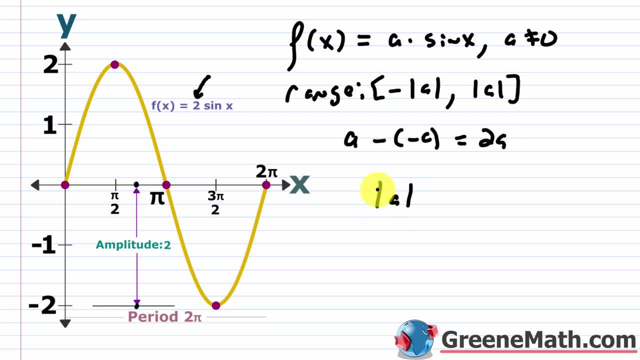 that I just get a And of course we're going to use absolute value bars just to account for the fact that this guy could be positive. It could be negative, So we want to account for that. So we use absolute value bars. So your amplitude- I'm just going to put amp- is always found as the 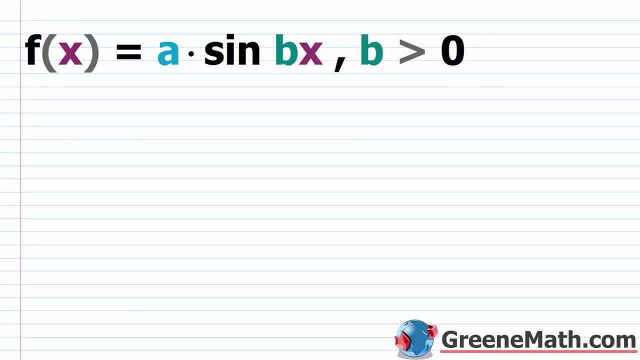 absolute value of a This guy out in front. All right. What I want to do is consider when the period for sine or cosine is not 2pi. I'm going to work with the sine function, but this works the same for the. 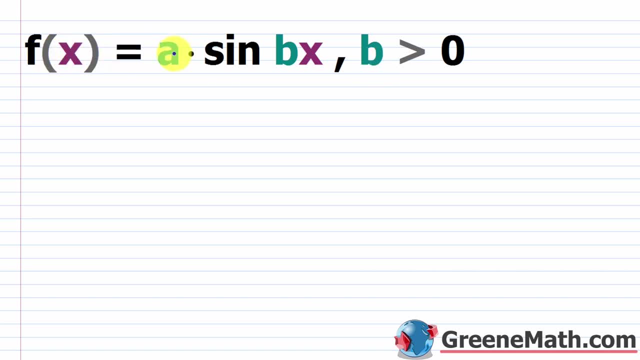 cosine function. So we have something like f of x equals a times the sine of. now we have bx, And I'm specifically going to work with b being greater than 0 in our examples today. You might get examples where b is less than 0.. I'll talk about how to deal with that. 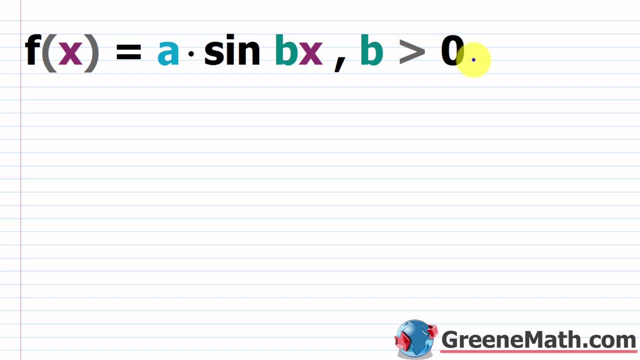 But we're not going to get to that scenario until the next chapter. OK, so I'm going to put a comma here. I'm also going to say that a is not equal to 0.. So any real number that's not 0.. 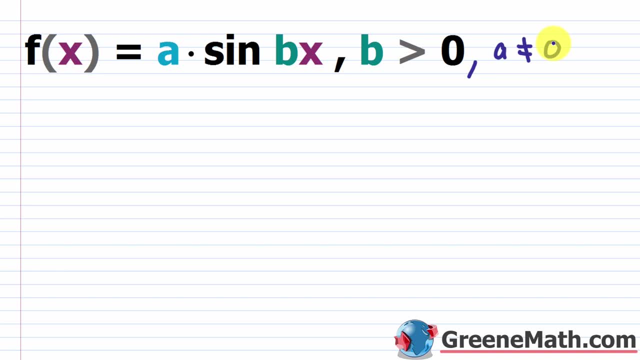 So, in order to consider how this is going to change our graph and how this is going to change our period, I want you to first consider that if b is 1, that's what we've been working with- So f of x is equal to a multiplied by the sine of x. This has a default period, So this has a. 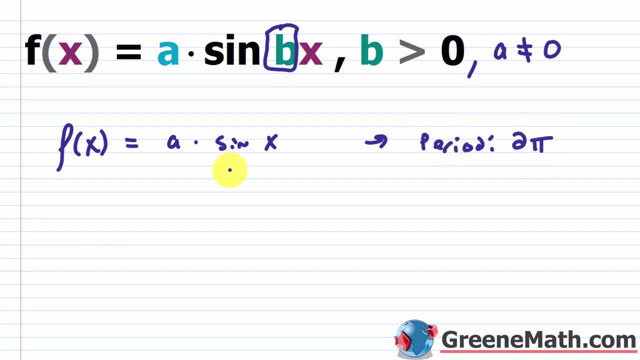 default period of 2pi. OK, now, where does that come from? Well, it comes from the fact that, as you rotate on your unit circle, starting at an angle measure of 0 in terms of radians, around one rotation, going counterclockwise to complete that rotation, you end up with an angle measure of 2pi. 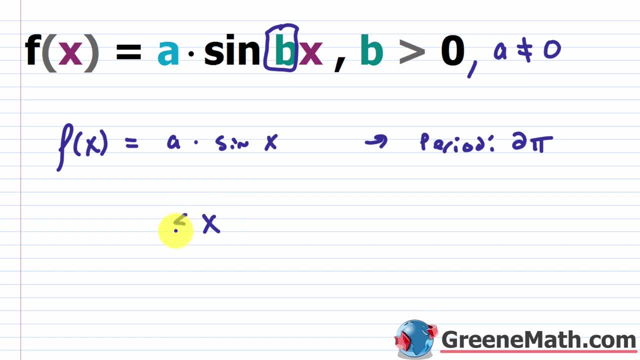 OK, so that's one cycle. So we would say: x is going to be greater than or equal to 0 and less than or equal to 2pi. OK, so this is what happens. as long as you have this format, It does not. 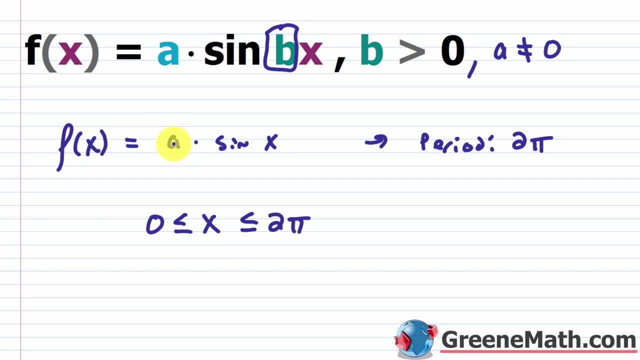 matter what the value for a is, Remember this is affecting us. with a vertical stretch or vertical compression, This could be negative. It could be positive. It could be negative. It could be negative. It could be positive. It could be negative. It could be positive. It could be negative, It could be. 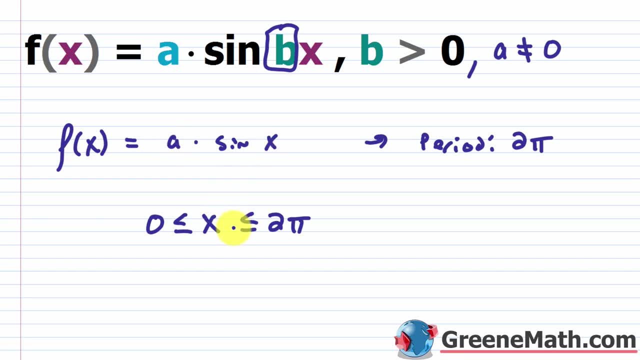 positive. It could be a fraction, It doesn't matter, It will not change your period. Now, when you consider that you're throwing this b into the mix, now something is multiplying x. OK, so it's changing the speed at which you're going through one cycle. OK, so you can throw this into your. 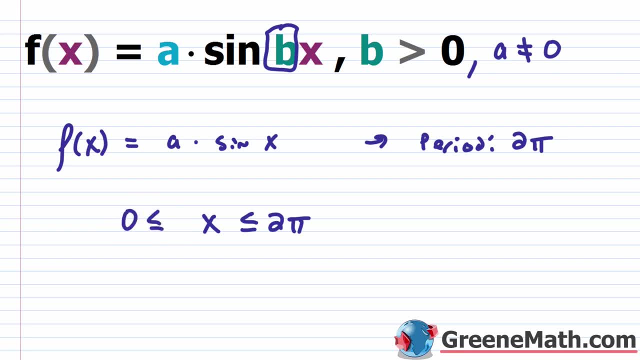 inequality. OK, and you can basically say that I'm going to put a bx inside of here, because my function is going to complete one cycle, as bx now increases from 0 to 2pi, So this might give you a horizontal stretch or horizontal compression. OK, it's going to change the speed at which you 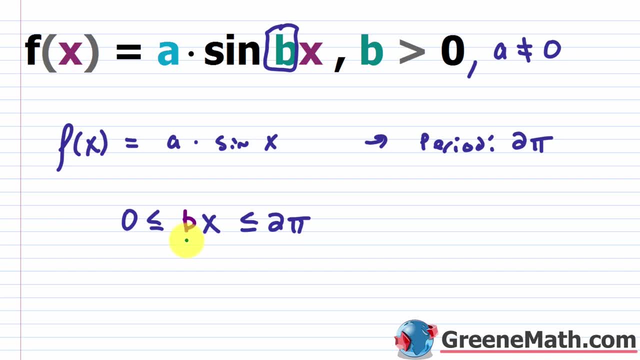 complete one cycle And basically to figure out what your period is, you're just going to divide everything here by b. OK, you're going to solve this for x 0 divided by b. Well, we know that b is not 0, so this would be 0.. OK, so let me write 0 here. This is less than or equal to, Well, the b's. 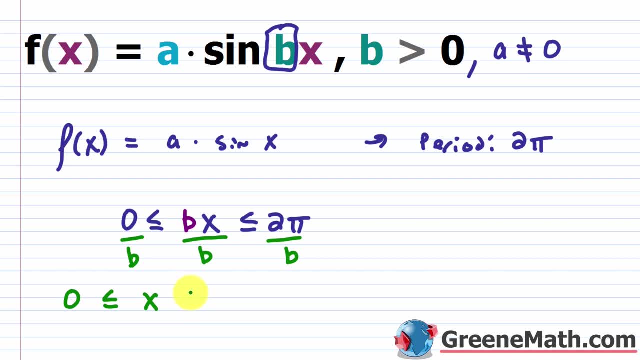 would just cancel out. b divided by b is 1.. So this is just x, And then this is less than or equal to your 2pi over b. OK, so we don't have any horizontal or horizontal compression, So we're. 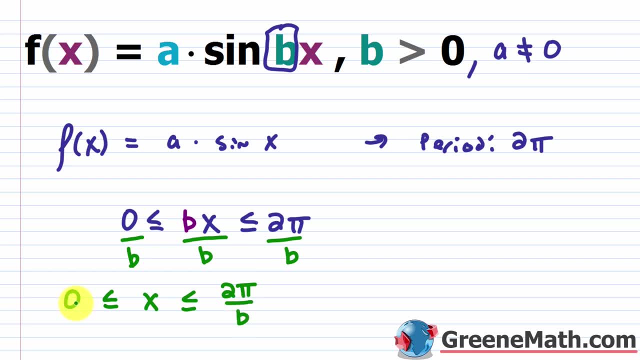 going to have vertical shifts going on. Your starting point for the cycle, OK, would still be 0 for the x value. And now your ending point for the cycle would be 2pi over b. OK, so we'll update the period and just put 2pi over b. OK, like that. And this is what you want to use as a general. 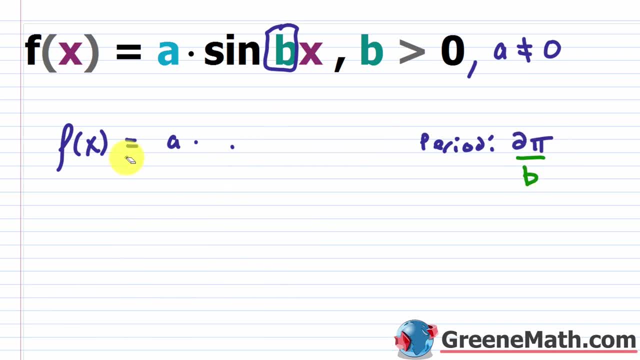 formula. OK, let me get rid of this And I want to talk about some other things. First and foremost, if you are in this section in your textbook and they are giving you problems, where b is negative, you can just use the absolute value bars for right now. When we get to the next, 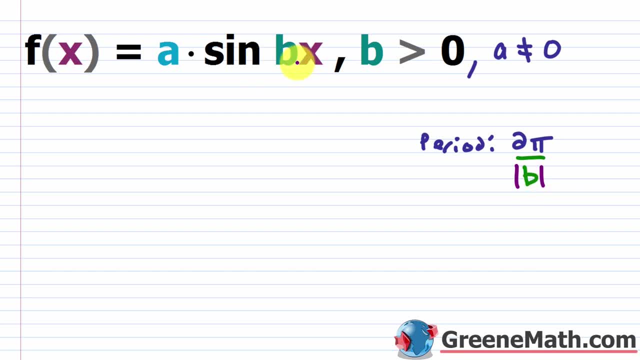 section. I'll show you how to rewrite this, based on the fact that sine is an odd function and cosine is an even function, to where b is always greater than 0.. OK, but for right now you can use the absolute value bars to get your period. Now, what I said earlier was that this: 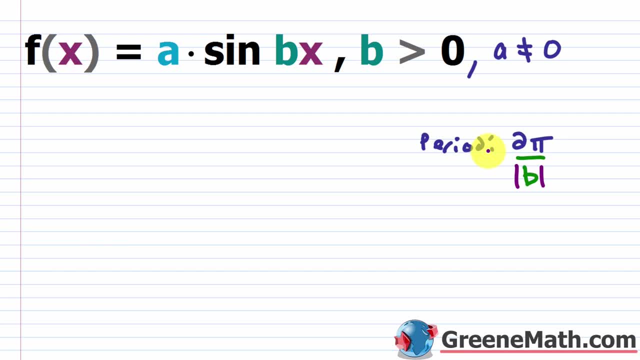 would create a horizontal stretch or a horizontal compression. Now where is that coming from? Let's think about a few basic examples. Let's say I said I had something like f of x is equal. to forget about the a, we'll just keep that as 1. each time I'll say the sine of 2x. Well, 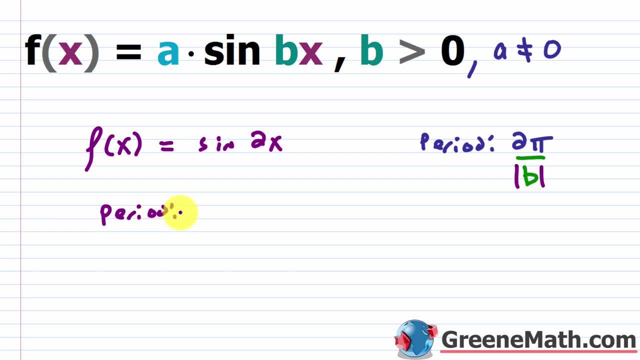 what about the period? So the period, OK, would be what? Well, I would have 2pi over my b value. This is my b value, It's the coefficient of x. So 2pi over 2, well, these are going to divide out. 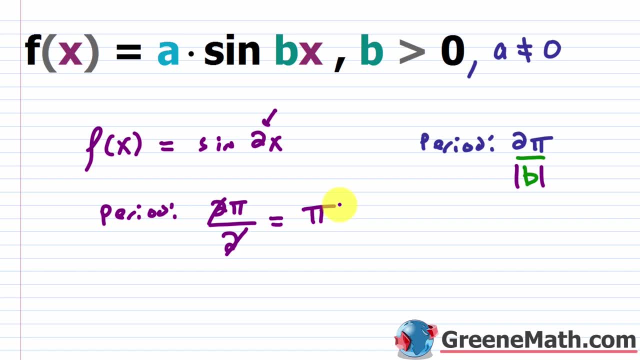 It's just pi. So if I think about this, it's completing a cycle OK, starting with an x value of 0 and ending with an x value of pi, versus normally starting with an x value of 0 and ending with an x value of 2pi. So it basically did it in half the time, right? So this is going to compress. 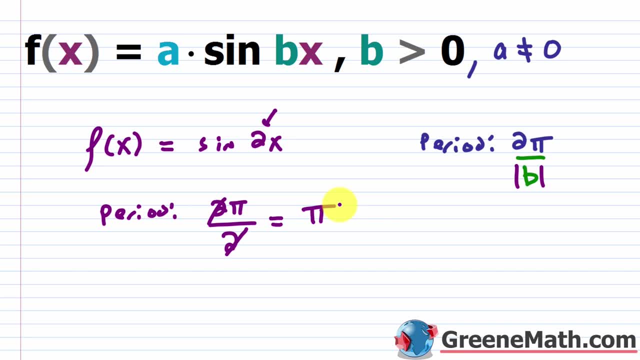 our graph horizontally. OK. So basically you can think about the fact that if your b is greater than 1, it is increasing the speed at which this bx here is going from 0 to 2pi. OK, So obviously that is giving me. 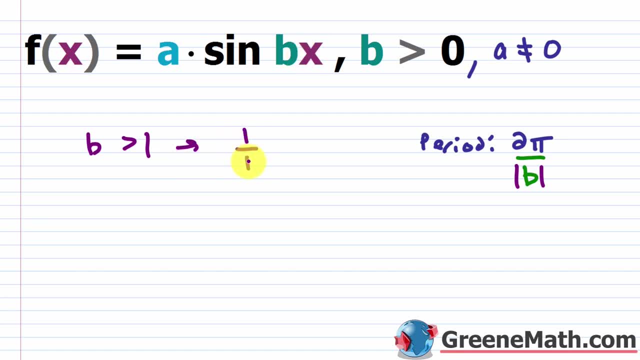 a horizontal compression by a factor of 1 over b. OK, So this is horizontally compressed by a factor of 1 over b. Let me erase this and let's talk about the next situation. So if this was a value between 0 and 1, so a fraction of 1 over b, then I would have a factor of 1 over b. 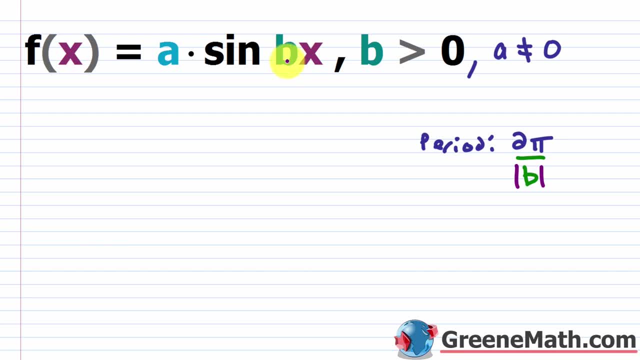 But now I have this very horizontal value. Now it's slowing it down. OK, So I'm going to be horizontally stretched. So let's say we looked at something like f of x is equal to. let's just do, let me keep my a value as 1, so I'll do sine of 1 half times x. Well, 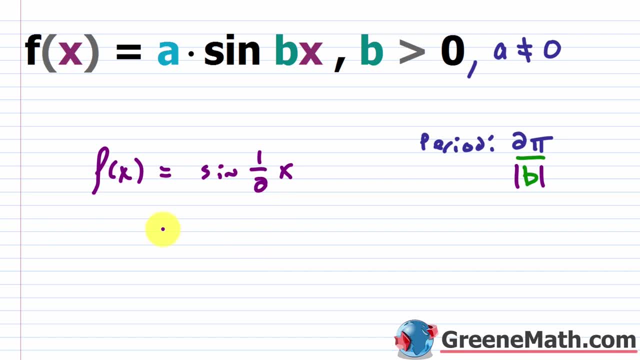 basically, this is going to stretch me out, OK, by a factor of 1 over. You would take this 1 half here. OK, So you're going to flip this and this is going to be 2, OK, So it's. 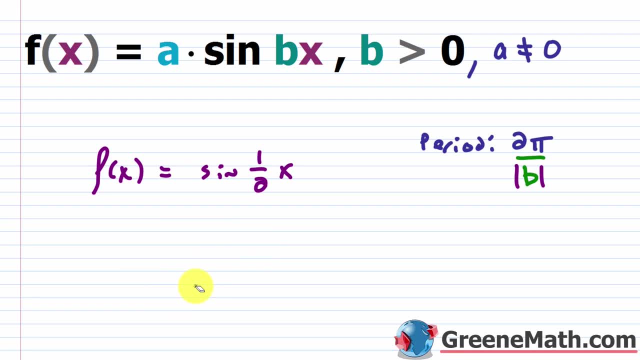 going to stretch me out by a factor of 2.. Again, to think about this with the period, your period is 1 over 0, x, x, y. So you actually get an x value of 1 over b. OK, So the fact, 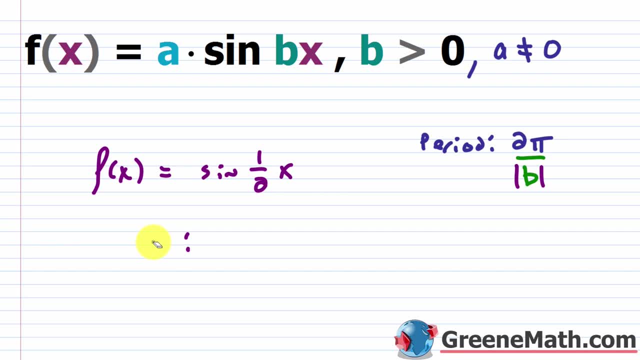 is always going to be, and I probably didn't write that correctly, so let me put this back in here. so the period would be 2 pi over b. now, if I'm dividing by half, I might as well just multiply by 2, so this is just going to be 4 pi, okay. so before it went from 0 to 2 pi, now it's going from 0 to 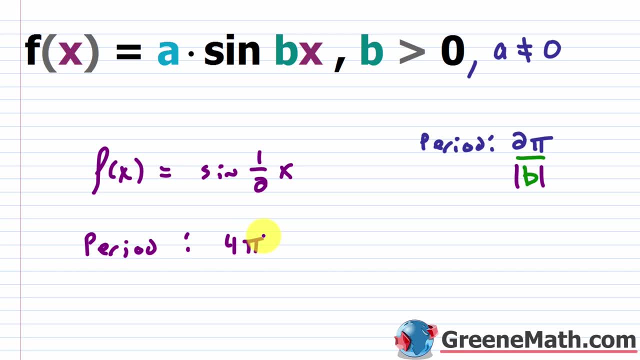 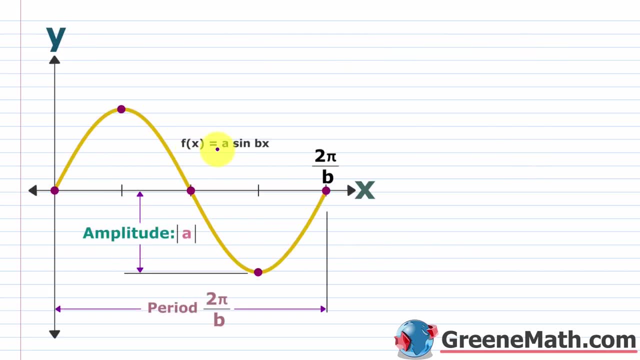 4 pi. so that is stretching the graph horizontally right. it's taking twice as long. so let's look at a simple little diagram here. I think this will make a little bit of sense for you. so we have f of x equals a times the sine of bx. again, we don't have any vertical or horizontal shifts, so the 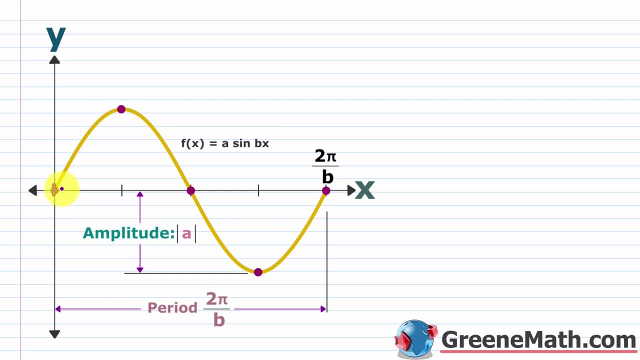 starting x value for your cycle is going to be at 0, and then you would add quarter periods- okay- to get these other notches. so you have your 2 pi over b. you'd multiply by a fourth to get your quarter periods. so you can cancel this with this, okay, and basically it's going to be pi over 2b. okay, that's. 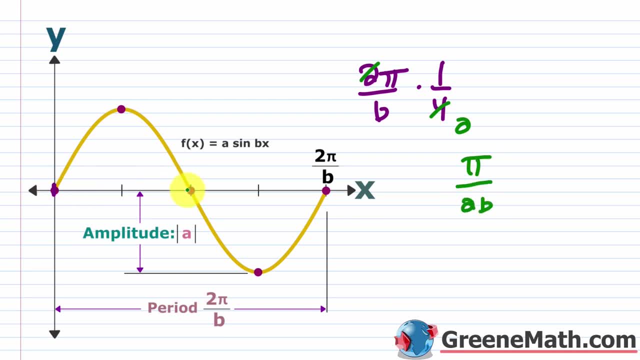 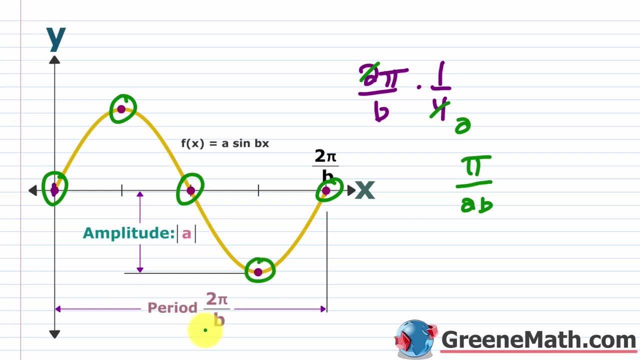 and your minimum, and you can get those from your amplitude, which is the absolute value of a right there. okay, your maximum is going to occur at the absolute value of that guy and then the minimum is going to occur at the negative of the absolute value of that guy. all right, let's look at two. 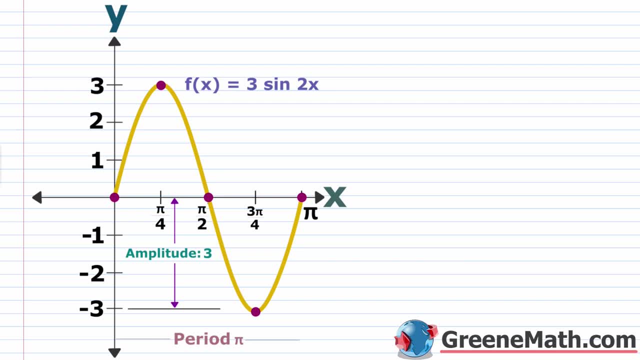 examples here real quick. I'll give you one where there's a horizontal compression and then I'll give you one where there's a horizontal stretch. so we have f of x equals 3 times the sine of 2x. so the first thing I'd like to do, if you're going to graph this, find your amplitude. okay, this is: 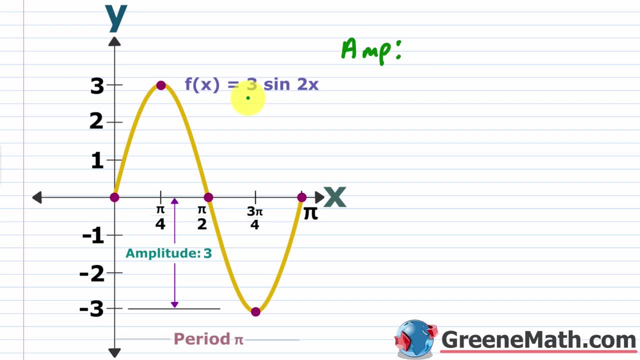 going to help you to figure out what's the maximum and the minimum. so this guy again: if this is 3, it's always the absolute value of that number, so it's going to be 3, okay, then find your period. so what is the period here? it's 2 pi over b. in this case, your b value is 2, so 2 pi over 2.. So this is just. 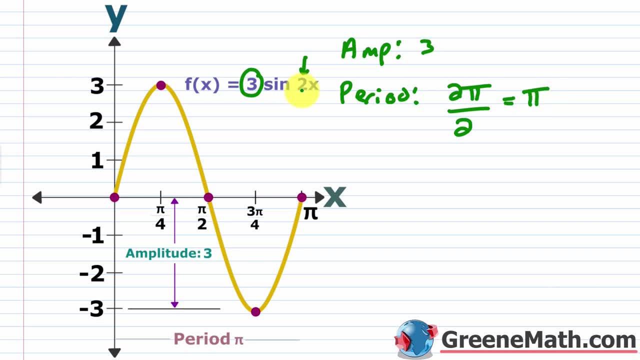 going to be pi. okay, so we know, because this guy right here, this 2 is greater than 1, because over here, this, we're going to have a horizontal compression by a factor of one over that number, so by a factor of one-half, And you can see, our starting x value is zero, our ending value is pi. so this is being completed. 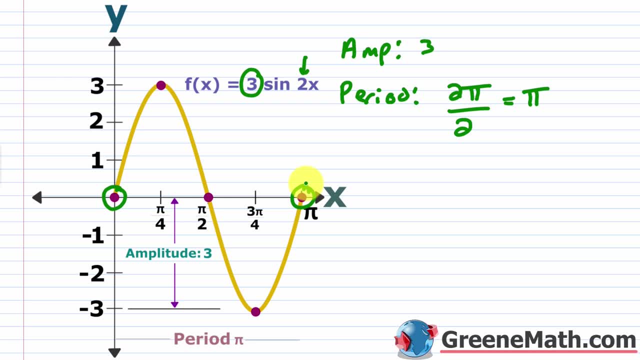 in terms of one cycle and half the time. So once you have those two things, you're going to go through and add these quarter periods. Let me erase this real quick and just put pi here. So a quarter period would be this guy divided by four, so it's pi over four. 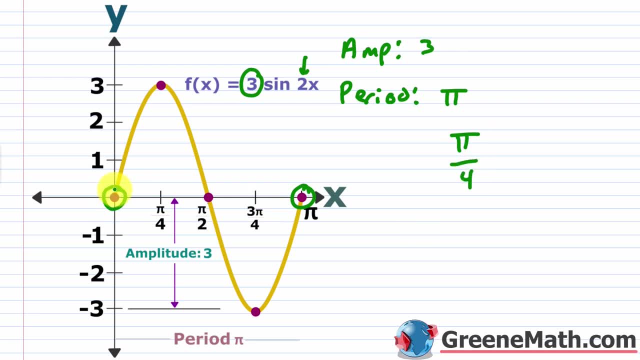 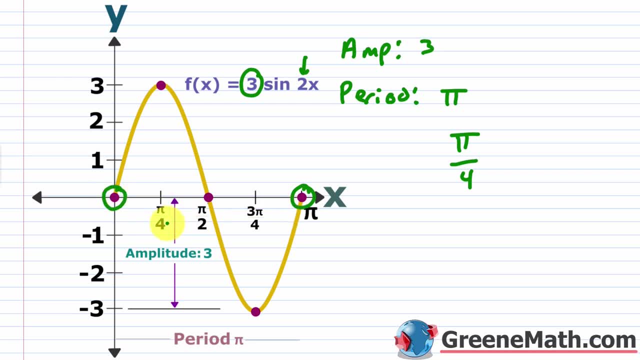 That's always something you check. I know it's not that important here, but when you get into things like a phase shift, which we'll talk about here shortly, it's going to be important to do that. So you have pi over four, you have pi over two, three pi over four and then pi. 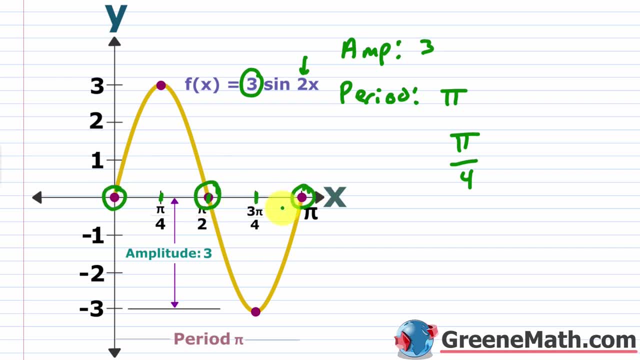 So you know that at the beginning, the middle and the end you have your x intercepts, so the y value is already figured out for you. it's going to be zero When you get to a quarter of the way through. and you get to three quarters of the way through. 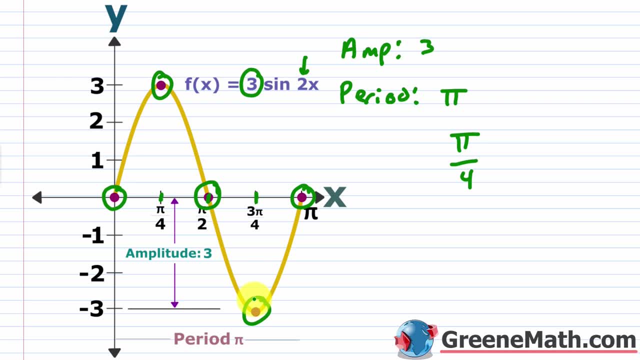 you know that you're going to be at your maximum for a quarter of the way through and your minimum for three-fourths of the way through and again from your amplitude. you know that's three. so the maximum's at three, that's your y value and your minimum is at negative three. 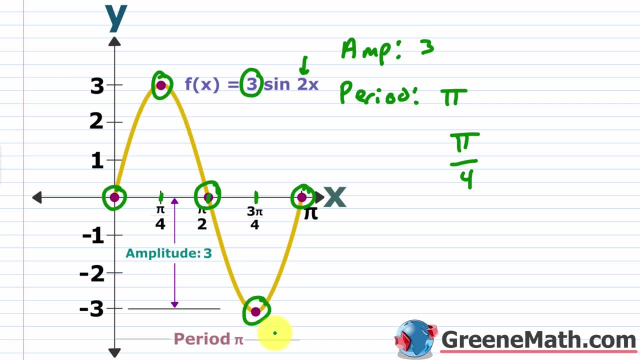 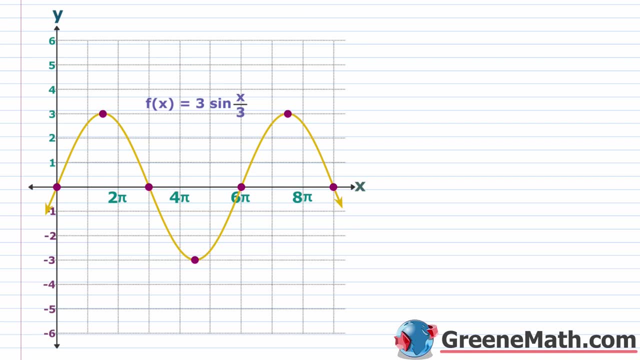 So that's enough to get you the five key points for this sine graph here and then just connect the points with a smooth sine graph. All right, let's look at an example now where we're going to have a horizontal stretch. So we're going to have f of x equals three times the sine of x over three, and you might. 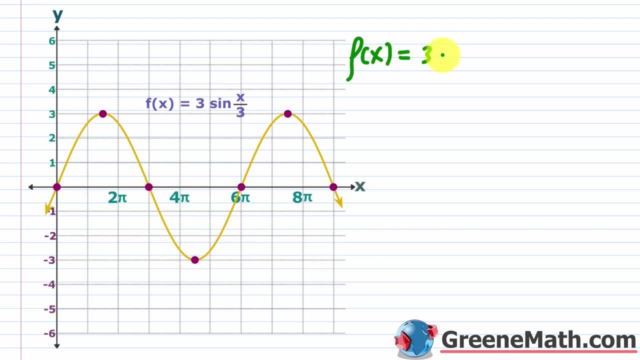 want to rewrite this. I'm going to go f of x is equal to. I'll put my three times my sine of- let me make that sine a little bit better- my sine of: instead of x over three, I'm going to put one-third being multiplied by x, like this. that way it's crystal clear. 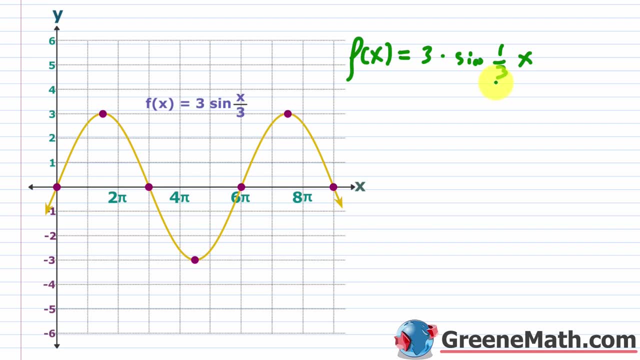 that the b value here is a third. Okay, So let's start off by thinking about our amplitude. so I'm going to put a m p for amplitude. obviously it's just the absolute value of this number. so again, it's just. 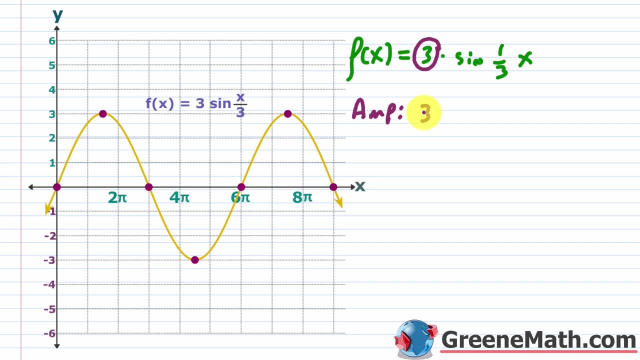 going to be three. Okay, So that tells me the maximum and the minimum. it's going to be three and negative three. right three for the maximum y value and then negative three for the minimum y value. Okay, Now, when we think about our period here. so when we think about our period, we're going 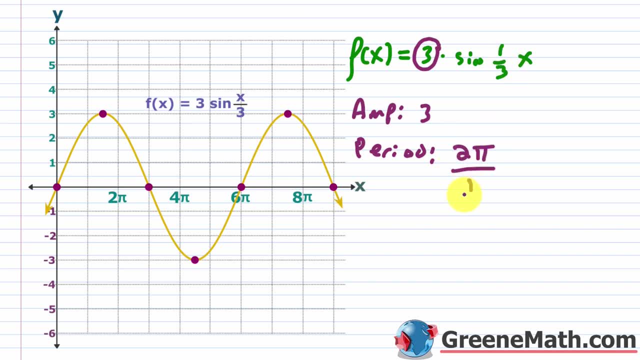 to have two pi over this b, So two pi divided by one-third. Basically, you're going to flip that fraction, okay, and you're going to have three over one and you're going to multiply that by two pi. so the period here is going to be six. 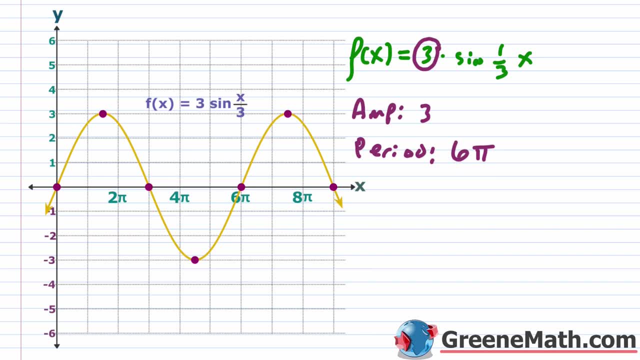 pi. Okay, So now, if we think about one cycle now, starting from this x value of zero out to this x value of six pi, so that's going to be one cycle for us, and essentially we can see that it takes longer to go through this cycle. right, instead of zero to two pi, now it's zero to 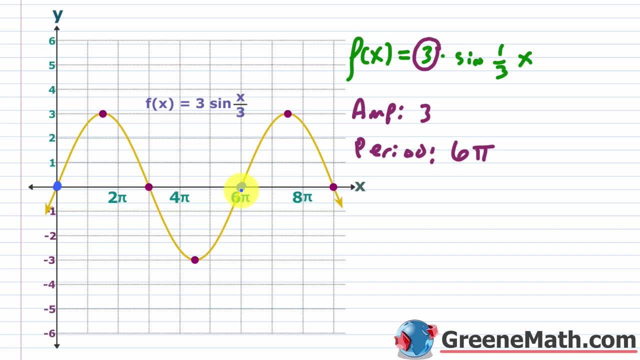 six pi. Okay, So what's happening is this is going to be a horizontal, So this is going to be a horizontal stretch of the graph. okay, by a factor. It's always by a factor of one over b. Here b is one-third, so one over one-third is equal to three. okay, so horizontally stretched. 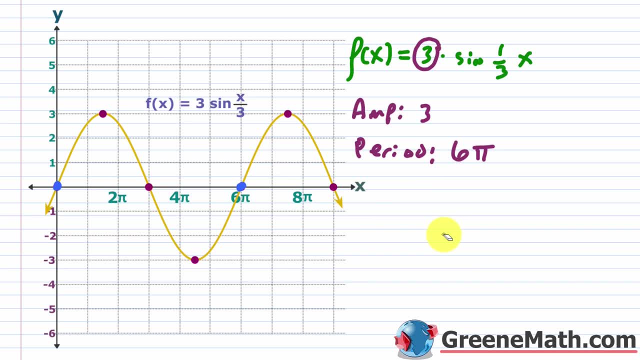 by a factor of three. Now, when we talk about sketching the graph of this guy, really all you need to do is get your key x values, okay. so you know this first one is going to be at zero and you know the y value there is going to be zero. 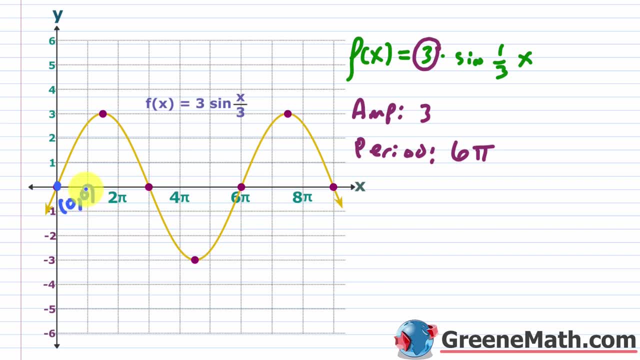 So this is zero comma zero. That's pretty easy to get From there. you want to add quarter periods, right? So you want to add quarter periods, right. So you want to add quarter periods, right. Okay, So you want to add quarter periods, right. 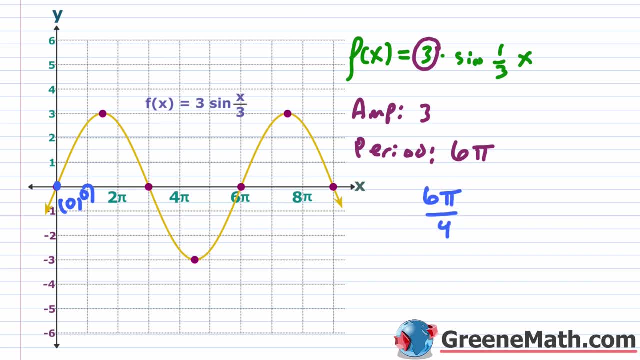 So you're going to go six pi over four. If I divide six by two, I get three. so let me write this as a three. If I divide four by two, I get two. so three pi over two is what I'm adding each time. 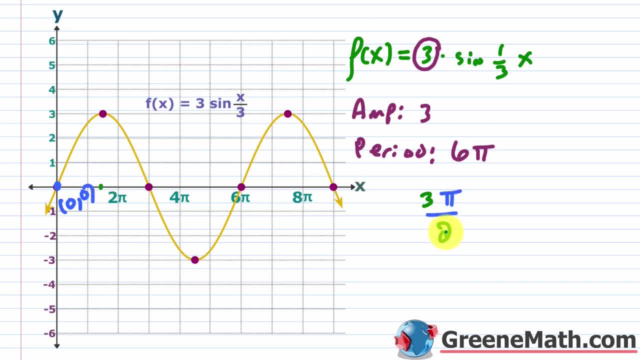 So basically, this notch right here would be an x value of three pi over two. so this point up here would be three pi over two, and then I'm going to be at the maximum, which is three. okay, So always when this guy is positive I don't have any kind of reflection or anything like. 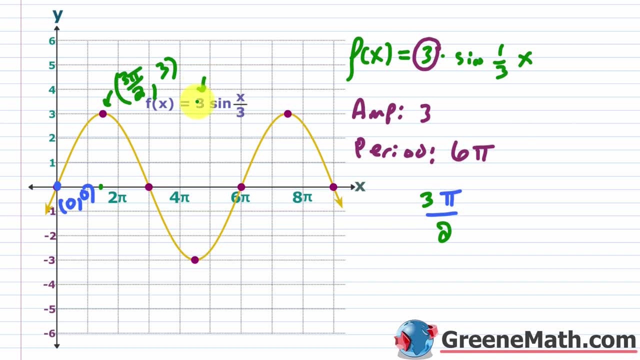 that I don't know how early we would reflect across the x-axis if this was a negative three. I know that a quarter way through I'm going to be at the maximum. okay, Because this is positive three. Now, halfway through, right here, I'm going to be back to my x-intercept. 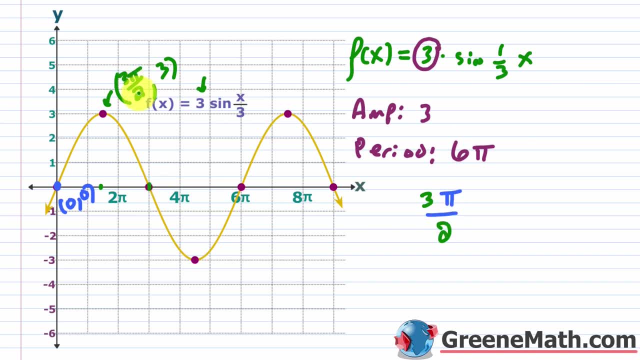 So to get that, I'm just going to add another three pi over two to my three pi over two. That would give me three pi, right? So this point right here would be three pi comma zero. okay, It's another x-intercept. 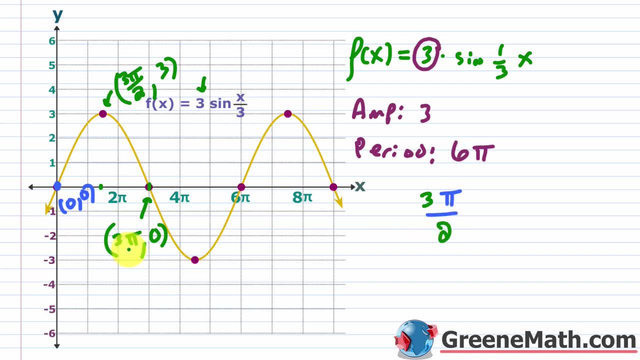 Then I'm going to add another three pi over two to this. So that's going to give me Nine pi over two. okay, so that's going to be my guy right here. So this point right here would be: nine pi over two and then comma. you're going to. 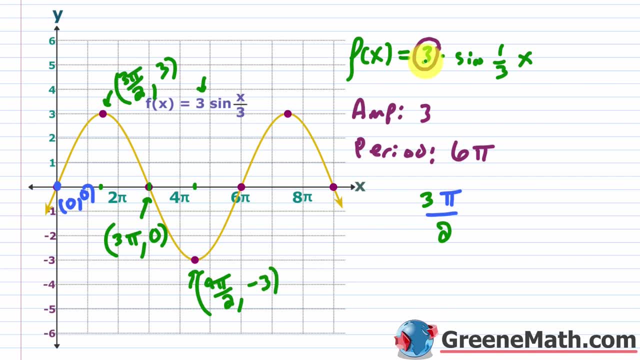 be at your minimum here, that would be negative three. So again, as long as this is positive here, your minimum is going to occur three quarters of the way through. okay, Again, if you get a negative here, you got to reflect across the x-axis, so you got to. 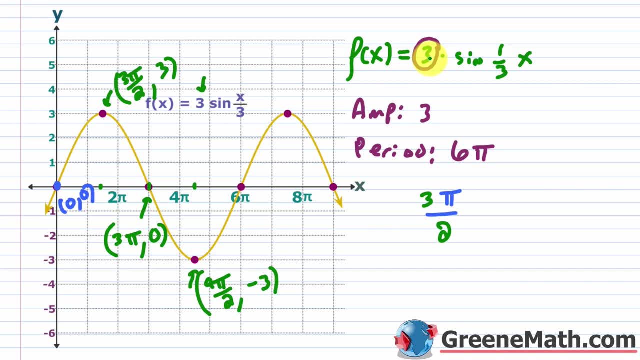 keep that in mind. okay, For right now this guy is positive, so it's pretty easy. Then you add another three pi over two to this nine pi over two and you're going to get your final x value of six pi. 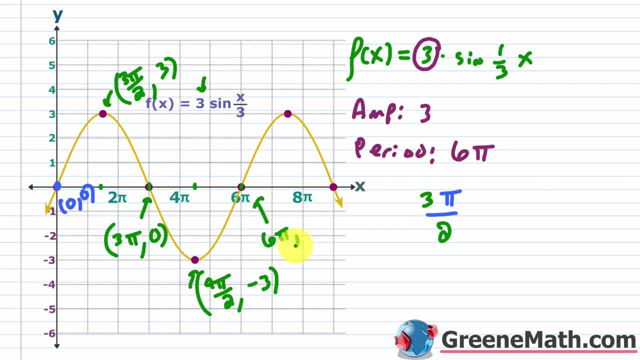 And of course this is another x-intercept. So this is six pi comma zero. okay, So once you get these five key points, this is enough to sketch one period of any sine function. So again, you're just going to connect the points with a smooth sine wave. 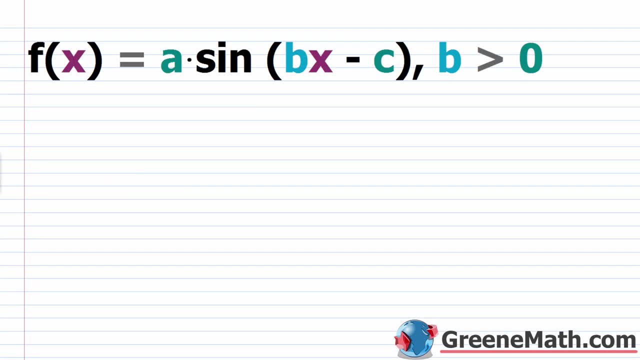 All right, so we have two transformations left that we want to talk about. One is going to be a horizontal shift, so either shifting to the left or the right. When we talk about this with the circular functions like sine or cosine, this is called. 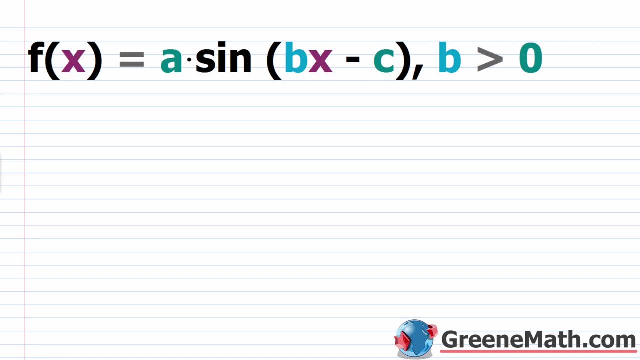 a phase shift. We also want to talk about a vertical shift, So shifting up or down, that's a lot easier to deal with, So we'll deal with that in a moment. okay, So right now we're going to look at f of x equals the a times the sine of you're going. 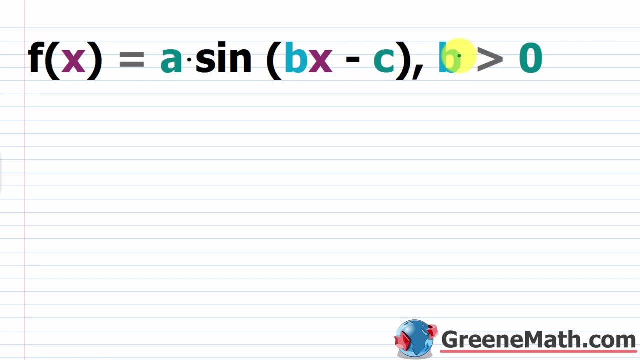 to have this bx minus c inside of parentheses And for right now, we're going to work with examples where b is greater than zero, just to keep things simple. Again, as we get into the next chapter, I'll talk about what to do when b is less than. 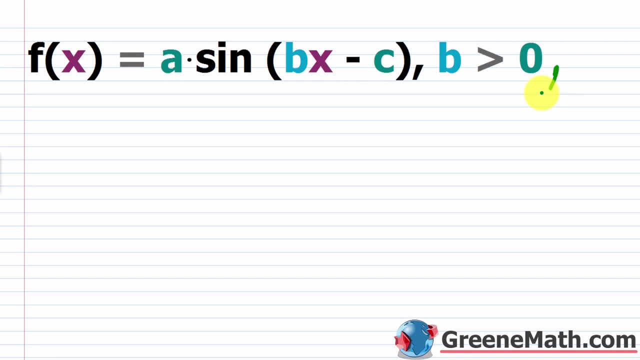 zero. And also, what I'm going to do here is I'm going to say that a is not equal to zero. That should be obvious, But I want to list that as a restriction, just so it's clear. So let's do that. 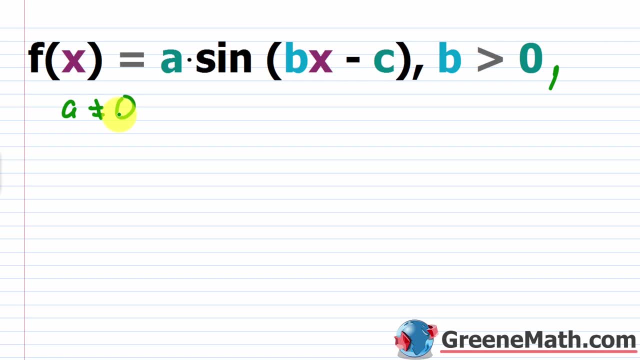 Okay, Now, when we talk about the phase shift, I want to first go back to something we learned a long time ago, just to jog your memory, So you know, if you have something like f of x is equal to, let's say, the square root, 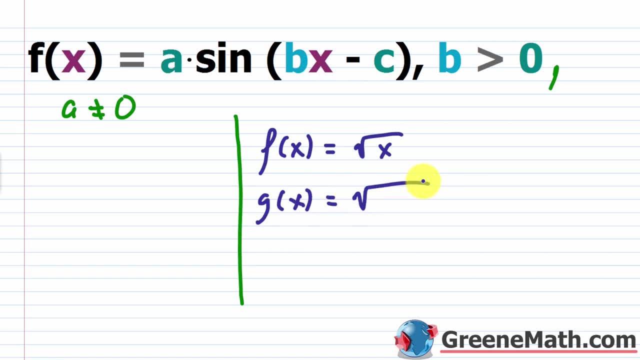 of x and you compare that to g of x, which is equal to the square root of. let's go x minus 2,. let's go h of x. let's say: this is the square root of x plus 2, okay. 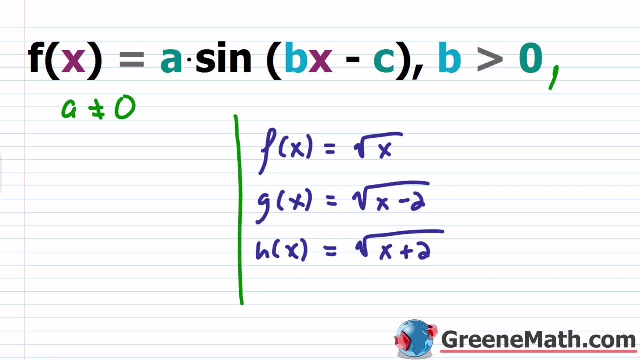 Remember, when things are happening inside the function, it's a little bit counterintuitive. right, When you see x values, you're thinking horizontal axis, so I'm moving left or right. When you see this minus 2,, most people assume that means that you have a shift based on this. 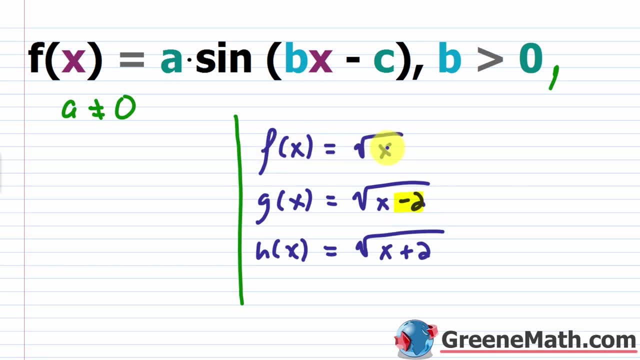 original graph f of x equals square root of x, that you're going to go two units to the left, But in fact it's the opposite. This guy is going to shift. This would shift two units to the right. okay. 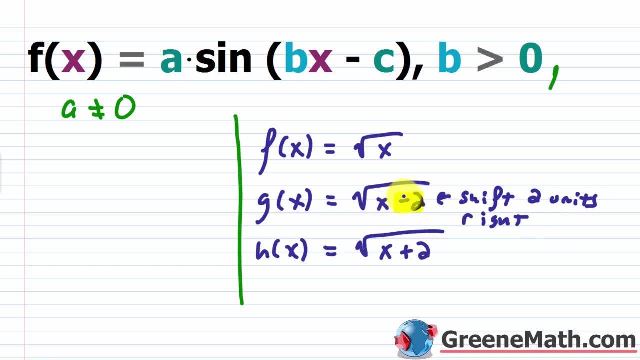 Now, what causes that? Well, you have to think about the fact that to undo what's being done to x, we've got to add 2, right, That gets me back to where I was, In other words, one ordered pair. 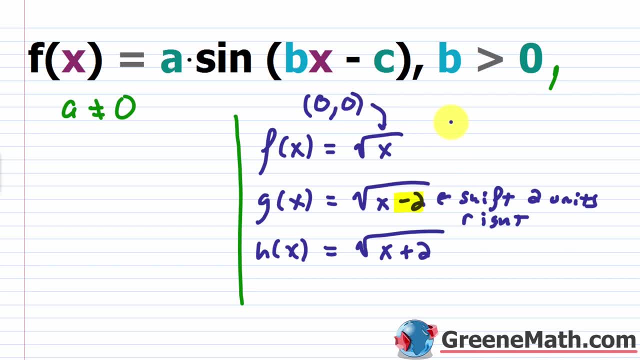 Let's say 0, 0.. That's on this guy. To get the same y value for this guy, the x value has to be two units larger, So it would have to be 2, 0,. okay, If you wanted to do another one, let's say you did for this guy something like 9, 3,. 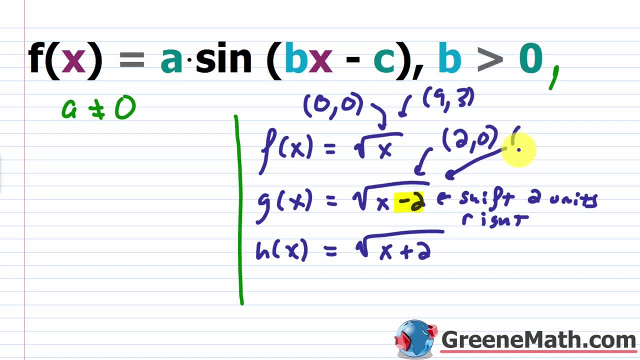 okay For this guy. again, the x value has to be two units larger, So now it would have to be 11, 3,. okay, Because you've got to go 11 minus 2 to get to 9, and then square root of 9 would get. 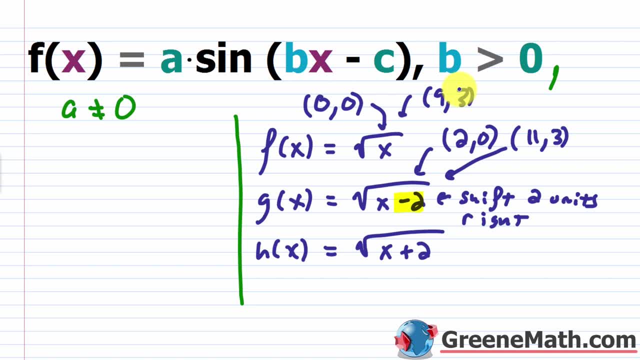 you that 3.. Here it's just square root of 9, which is 3.. If you look at this guy again, what's being done? I'm adding 2, so to undo that I've got to subtract 2, so that means I'm shifting. 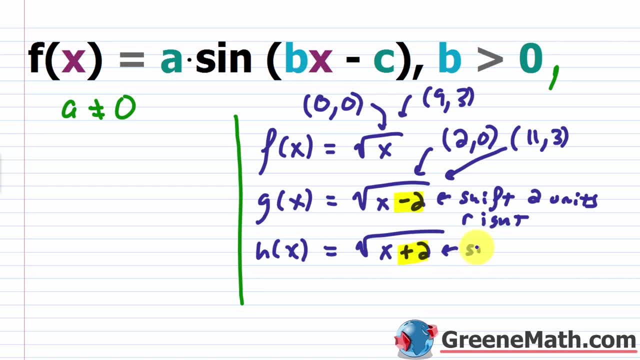 two units to the left. So I'm going to let me change my marker here. I'm going to shift two units left, okay? So you've got to keep that straight in your mind. It's the opposite of what you think, right? 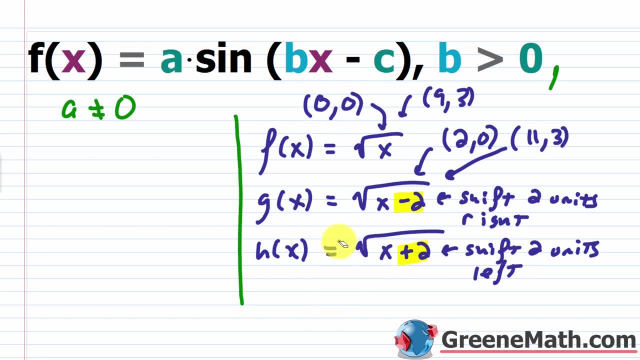 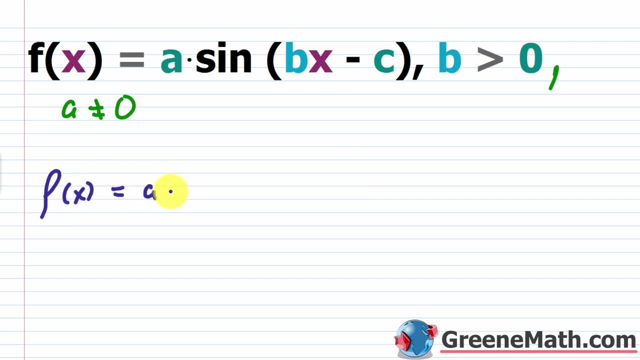 You've got to undo what's being done to x. Now let me erase this, and what I'm going to do is I'm going to write this in a different way. okay, So I'm going to write: f of x is equal to a times the sine of. 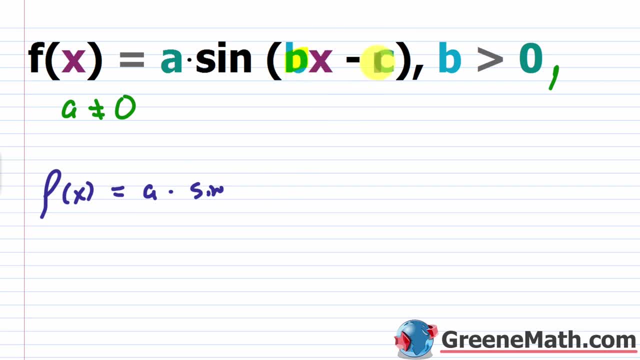 I'm going to factor this b out. Now you might be saying: well, there's no b over here, so how are you going to do that? All you need to do if you want to factor that out is basically divide each term by b. 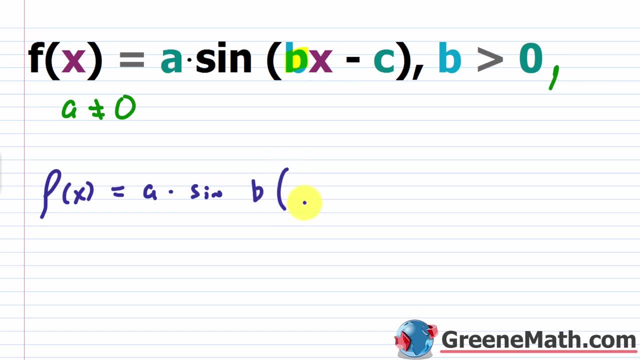 So, in other words, I can put a, b out here and then, inside the parentheses, I can go ahead and say: well, bx divided by b is x, and then, minus vc, divided by b, would be c over b. okay, So this is going to make your shift a lot more clear. 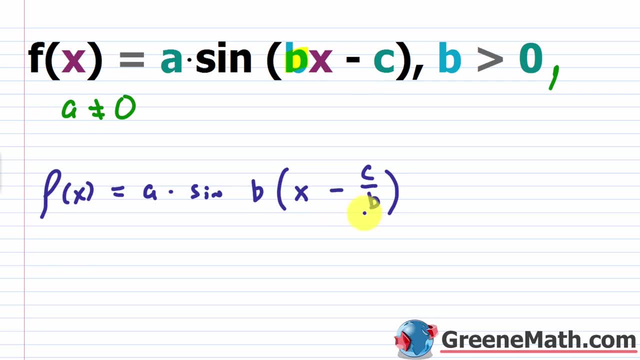 You can do it from this form if you want. Most people do, But I advise, if you're having trouble with this, So write it like this: I can also say that a is not equal to zero and I can say that b is greater than zero. 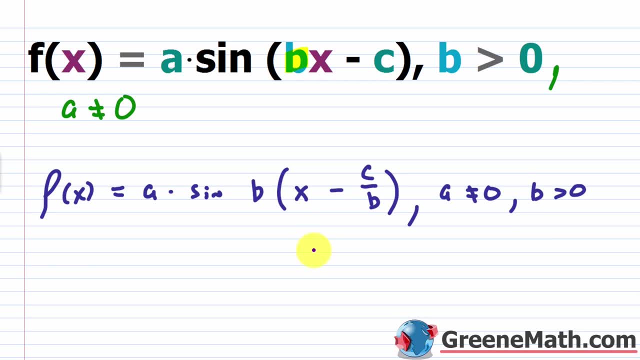 for our examples, And you might want to make this crystal clear and put some brackets here. They're not needed, but that makes it a little bit cleaner, okay. So if I look at it in this form, I know that if c is positive and b is positive, that basically. 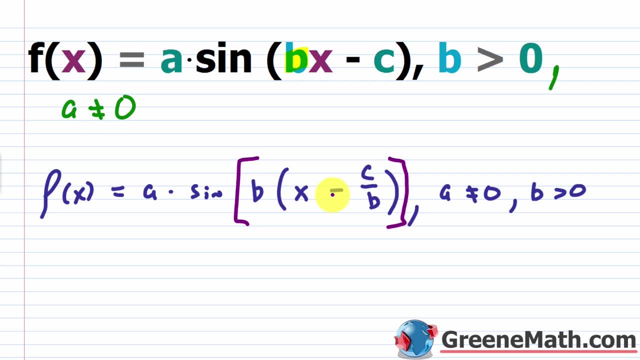 I'm subtracting away a positive number, okay, And I'm going to be shifting to the right by c over b units, okay, It's very, very simple, Okay. So if, for example, this was a negative c, I know b is positive because I've made it. 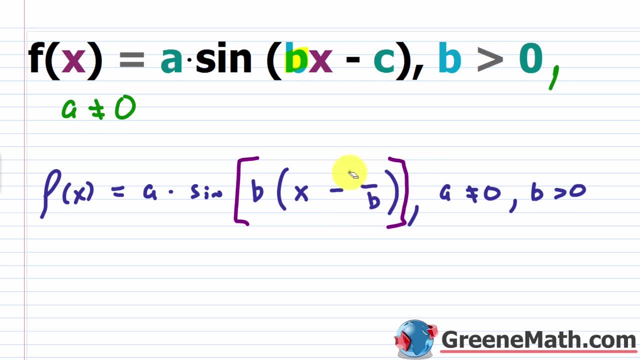 that way. Well then you have minus a negative, which is plus a positive, right? So I could really write this as plus c over b. In this case I'm going to shift to the left. okay, by c over b units. or you could say: 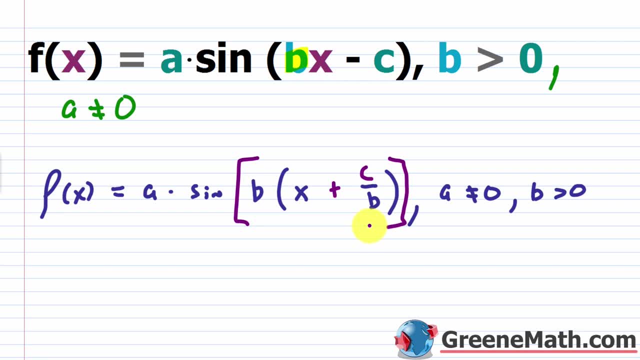 really to make that crystal clear, since I said that c was negative by the absolute value of c over b units. okay, to make that crystal clear, Let's put this back to this original form Now, if you want to work with it in this form, it's really the same thing. 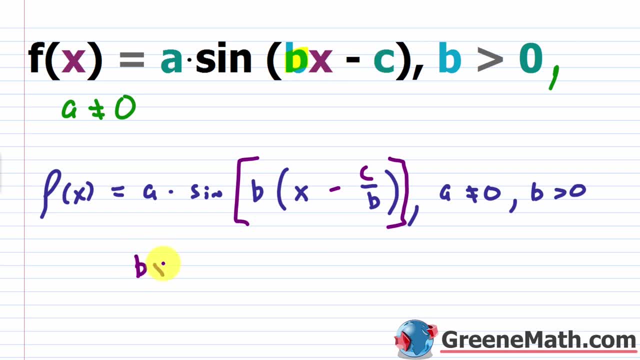 Okay, All you would do is start off with bx minus c and you could set that equal to zero and you could say: well, how do I undo what's being done to x? Well, what I could do is I could add c to both sides. okay. 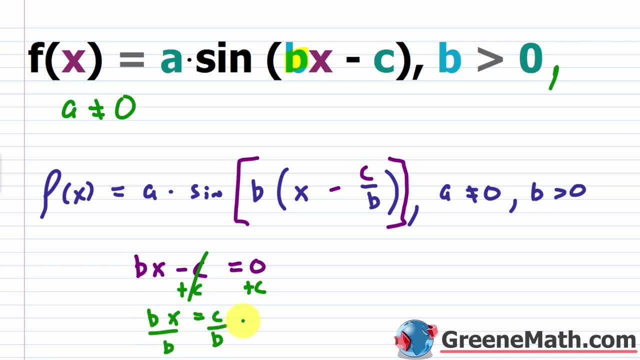 Cancel that and say: I have bx is equal to c. divide both sides by b and I'll say I have x is equal to c over b. So that's going to be your phase shift, okay, Again, dealing with whether it's going left or right is just based on the sign that you 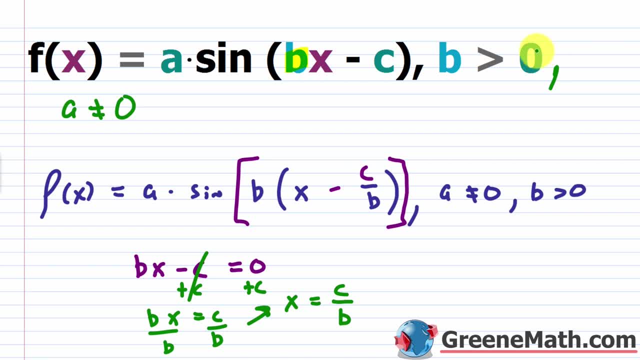 have If b, again, is restricted to be positive. Well then, If c is positive and you have it in this form, you're going to be shifting to the right by c over b units. okay, If c is negative, meaning you have plus a positive, you're going to go to the left by. 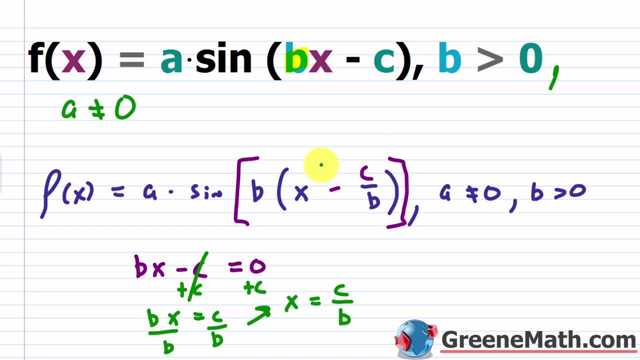 the absolute value of c over b units. okay, This one's a little bit tricky when you think about the signs, when you're in this generic form, So let's go ahead and look at an example. I think it'll be a little bit clearer. 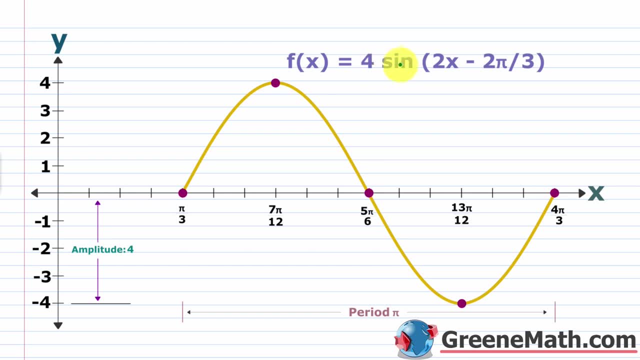 Okay. So let's look at this: f of x equals 4 times the sine of. we have the 2x minus 2 pi over 3.. So if you wanted to, you could rewrite this. I'll go. f of x is equal to, you'll go, 4 times the sine of. I would factor out the 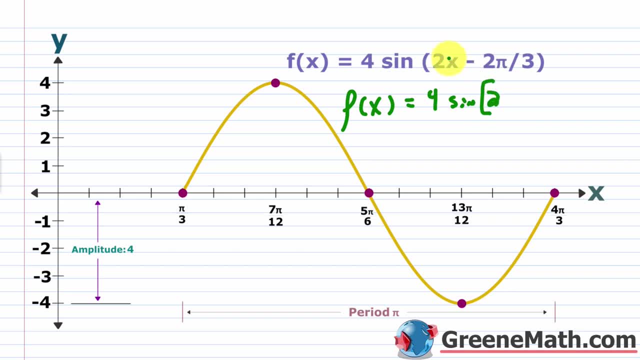 2,. okay, And I would put that out in front And then inside, you're going to divide everything by 2.. So if I divide 2x by 2, I get x And then minus. if I divide 2 pi over 3 by 2, it's like multiplying by a half. 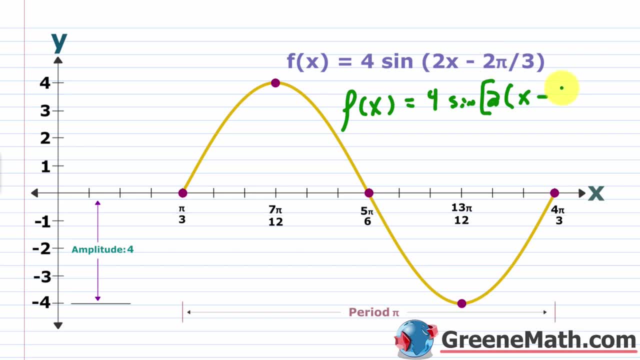 Basically, you would cancel that 2 out with the 2 in the denominator, So you would have your pi over 3, okay. So really, when you look at it, you can just go back to my simple example. with the square root You have this minus pi over 3.. 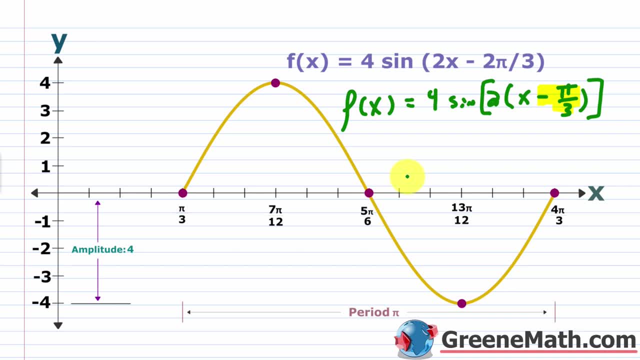 So your phase shift is just going to be pi over 3 units to the right. okay, If this was a plus here, I would be going pi over 3 units to the left. okay, That's how I would write it. It's the simplest way to do it. 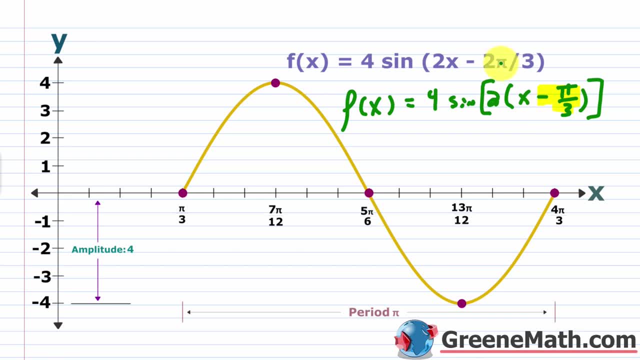 If you don't want to go through all this trouble of factoring it, you can always say that I want to do my phase shift as c over b. okay, So my c is going to be 2 pi over 3.. Let me write this out. 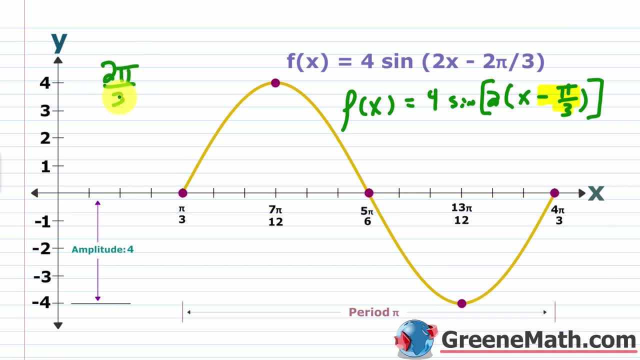 So my c is 2, pi over 3, and then divided by b, So I'm dividing by 2, okay, So it's like multiplying by a half and again this 2, we cancel with this 2, and you end. 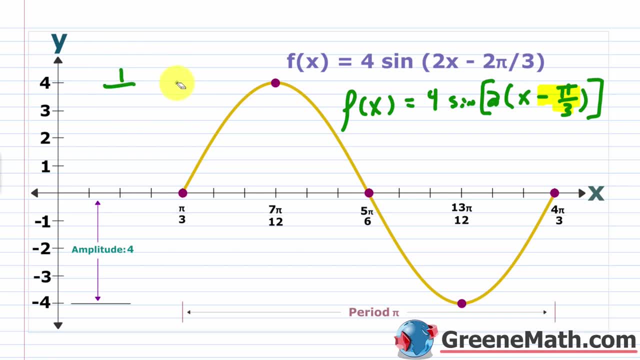 up with pi over 3.. And again, because this was positive here, what that means is that we're going to be shifting to the right by pi over 3 units. okay, So let me write out here that my phase shift is pi over 3, and this is to the right. 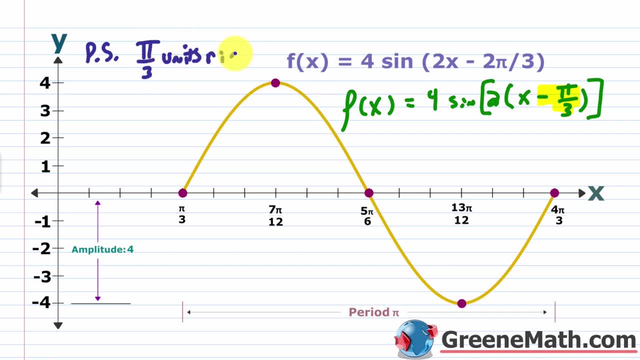 So pi over 3, you can put units if you want And you will put right, okay. So you can see that by looking at the graph. normally we start at 0, 0.. Now we've been shifted pi over 3 units to the right. 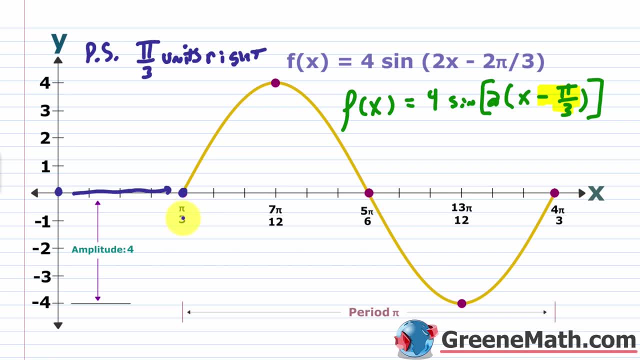 So the first guy for this cycle to start it off, the x value is pi over 3, and the y value is 0. So pi over 3,, 0,. okay, Now when we talk about the other five key x values, from this point it's the exact. 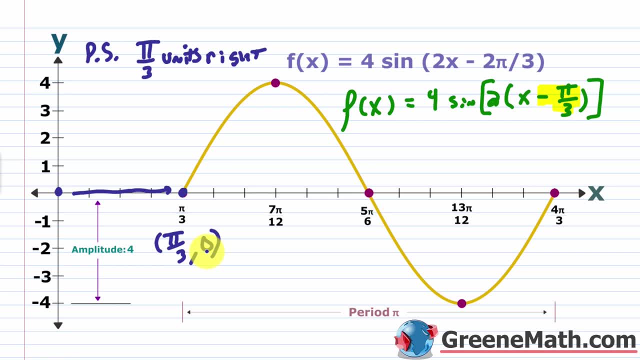 same procedure, okay. Same song and dance. So I'm going to find my amplitude again. that's super easy to do. Absolute value of this number out in front. so the absolute value of 4 is 4, okay, And this is not a negative, it's a positive. 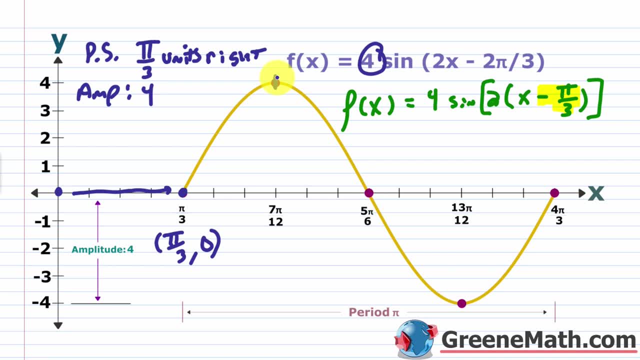 So you know your maximum is going to occur at the quarter way through the period. Your minimum is going to occur at three-fourths of the way through the period. So we'll get to that in a moment. But you know, basically the y value here would be 4, let me go ahead and write it out and 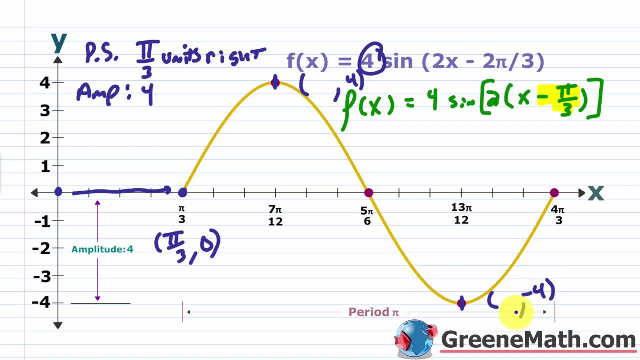 the y value here would be negative, 4, okay, So that's pretty easy. You also know that your y value at all your intercepts, okay, which is going to occur at the halfway point And at the ending point it's going to be 0.. 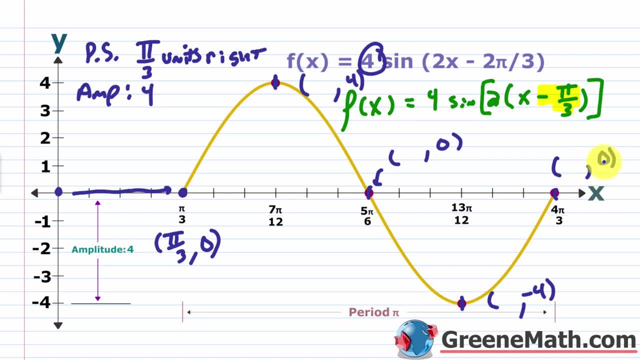 So that's pretty easy too. So let me go ahead and put those in Now. how do we get these x values? How do I get this one and this one and this one and this one? Again, you're just going to add quarter periods. 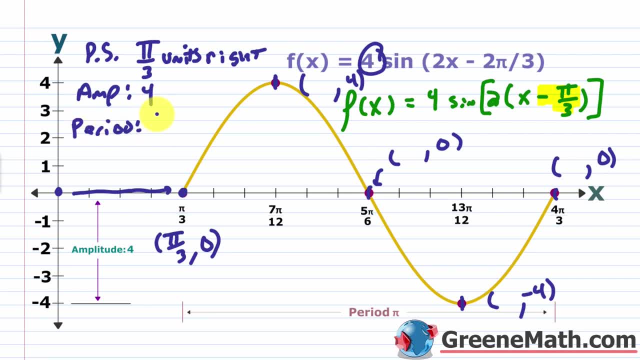 So we first need to find the period to do that. So let's go ahead and find the period And basically, if we look at it, we have a b value of 2.. So we have 2 pi over 2, which is just going to be pi, okay. 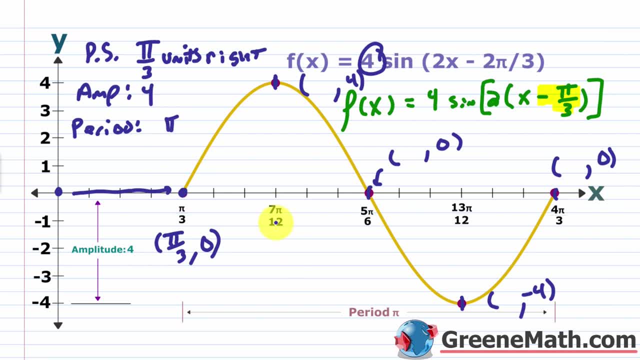 So if you wanted quarter periods, it's pi over 4.. So I'm going to add increments of pi over 4, okay, And you can see I already have this listed. This is something you would have to do with either a calculator or by hand. 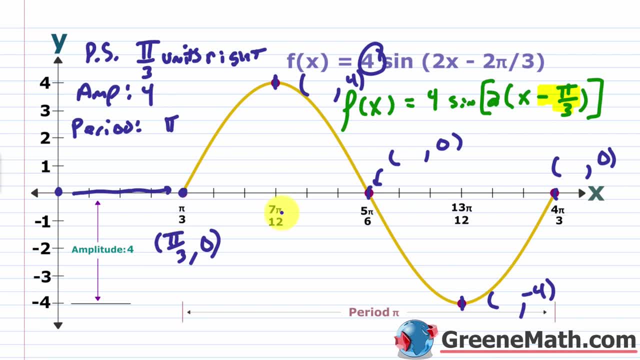 So basically, pi over 3 plus pi over 4 is going to give me this 7 pi over 12.. So this is 7 pi over 12.. Add pi over 4 again and I'm going to get this 5 pi over 6, so 5 pi over 6.. 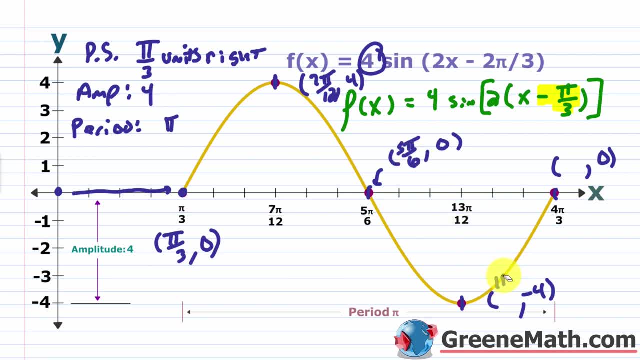 Add pi over 4 again. I'm going to get this 13 pi over 12.. So let me write that in there. So this is going to be 13 pi over 12.. And then add pi over 4 one more time and I'm going to get to 4 pi over 3, so 4 pi. 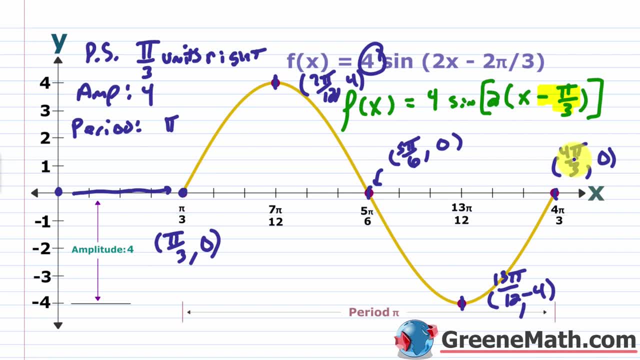 over 3.. I talked about this earlier and it might have not made sense at the time, but when you have a phase shift, you want to take this guy and this guy and you want to do a little subtraction to make sure it equals the period. 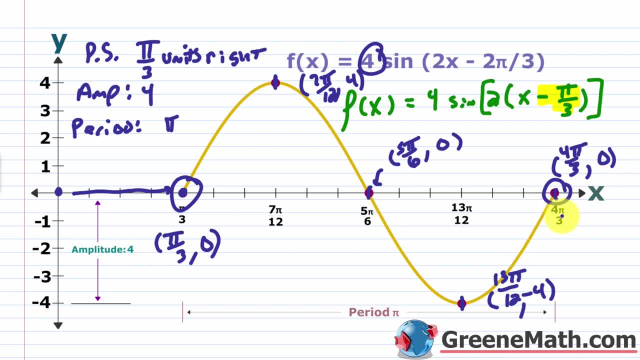 That way you know you didn't mess up when you were adding quarter periods. okay, So 4 pi over 3 minus pi over 3 does give me the period of pi. so I know I'm good to go right. I have all my points and then I can just sketch my graph by making a smooth sine wave. 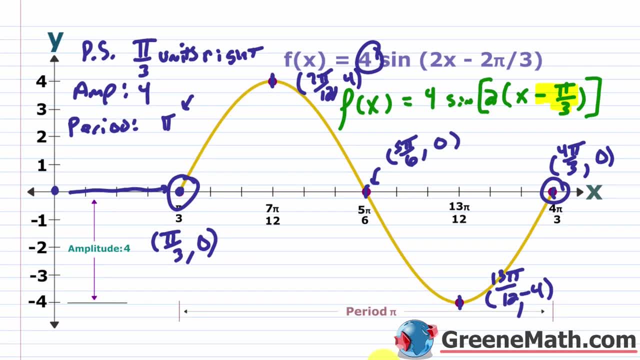 through those points. Now, if you wanted to think about all the transformations that have occurred, I'm going to write this down. Some teachers will ask you for that. Basically, you can think about: okay, it's been vertically stretched by a factor of 4.. 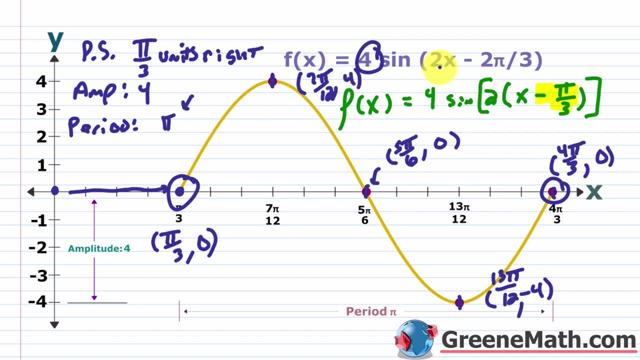 It's been horizontally compressed by a factor of a half right. So remember it's 1 over b. Your b value here is 2, so 1 over 2 or a half. okay, This guy is basically running through a cycle in half the time. 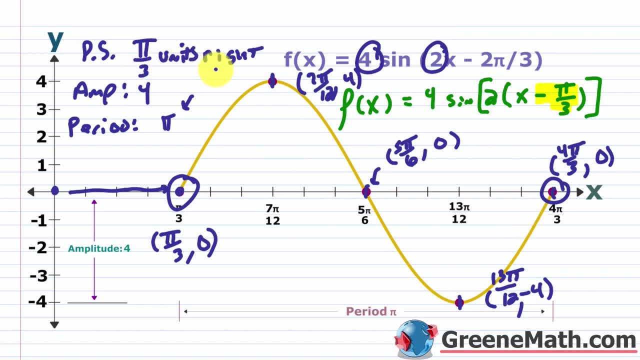 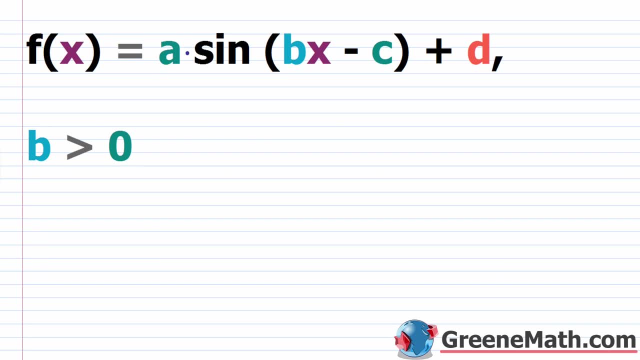 Your phase shift is going to be pi over 3 units to the right. All right, let's talk about the last graphing transformation, which is basically where we're going to shift up or down. Okay, We have something like: f of x equals a times the sine of bx minus c, and then plus d. now 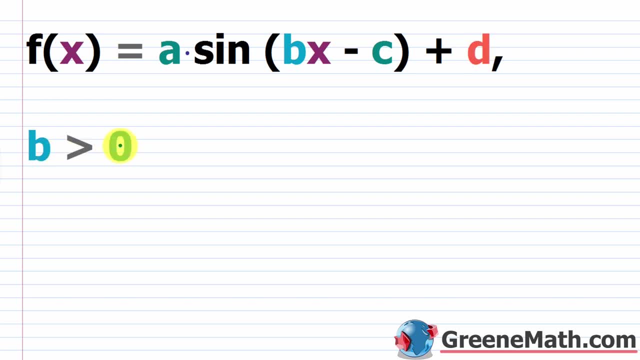 We're still going to say b is greater than 0.. Again, we're going to deal with b less than 0 in the next chapter and I'm going to specifically state that a is not allowed to be 0. This is just for clarity, okay. 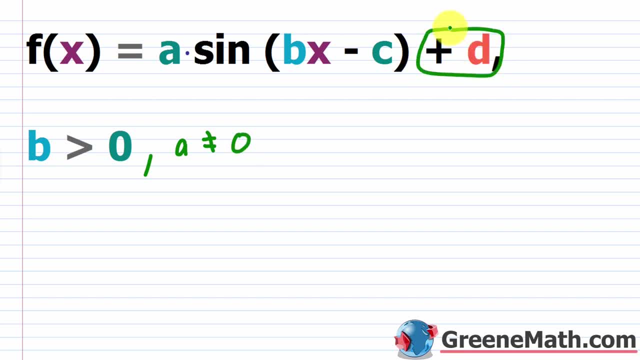 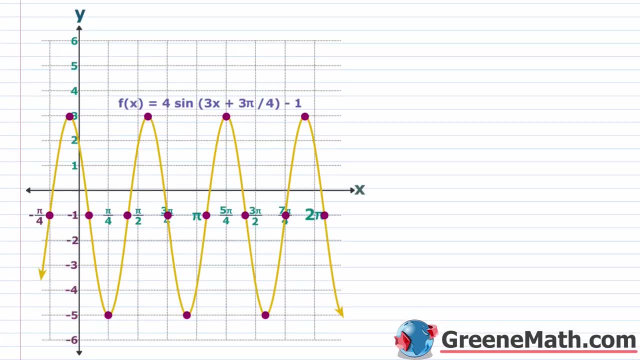 So here, because of this plus d, this is a vertical shift. You're going to go up by d units if d is positive. You're going to go down by the absolute value of d units if d is negative. Let's go ahead and look at an example. 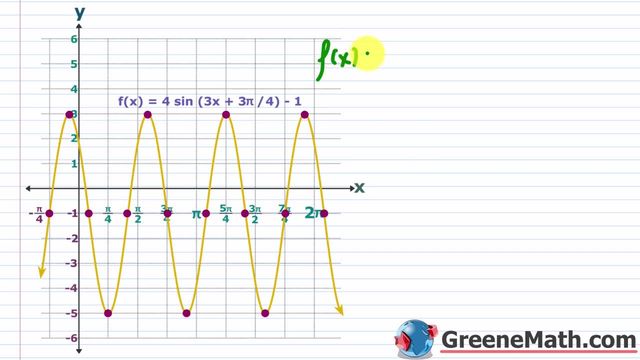 We have f of x equals 4.. Let me write this out here. So f of x equals 4, then multiplied by the sine of, You're going to have this 3x plus 3 pi over 4.. I'm going to factor that 3 out. 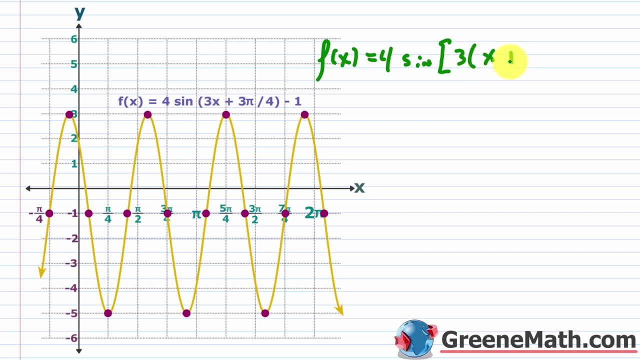 So inside, instead of 3x, I'm going to divide by 3.. I'm going to have x, then plus, Instead of 3, pi over 4, let me write this out so nobody gets lost: I'm going to divide. 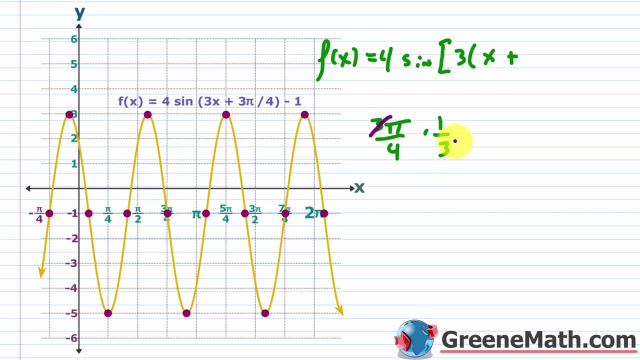 by 3.. So that's like multiplying by a third. So you're going to see that the 3s are going to cancel and you're going to have pi over 4 right here. Let's write that in, Close that down. 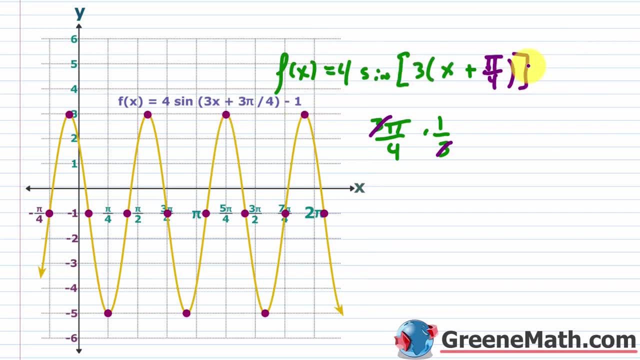 Let me scooch this over, so everything fits. You also have this minus 1 here, so we'll put that out there. If you were to think about this- let me make that a little bit cleaner- If you were to think about this in terms of all the things that have been done based on 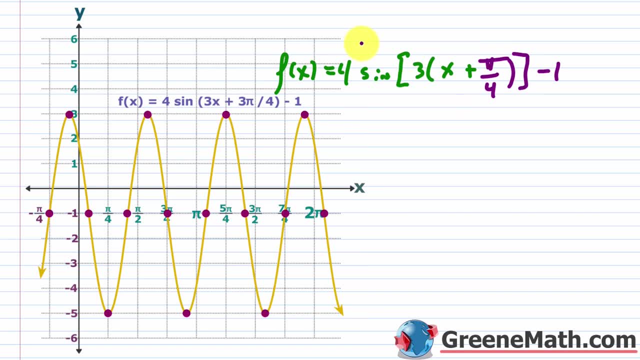 the original sine graph that we were working with. well, you have a vertical stretch by a factor of 4.. You have a horizontal compression by a factor of 1 third. So 1 over b- in this case b is 3.. 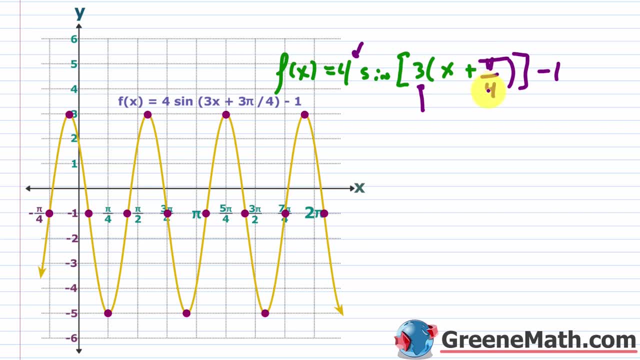 You have a phase shift left by pi over 4 units because you have x plus pi over 4 inside here. So you're going left by pi over 4 units And then you're going down by 1 unit. That's what that negative 1 is going to do. 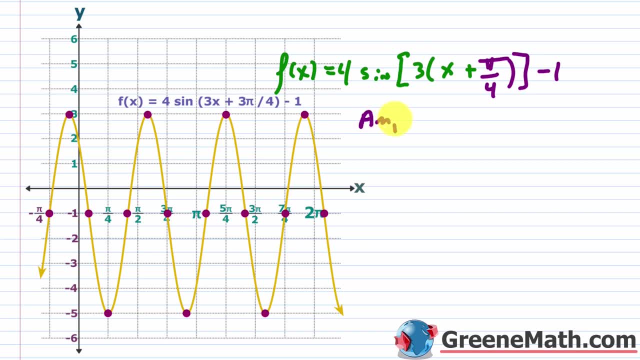 So if we think about this, we can get our amplitude Again. we know that that is going to come from this number. right here, The absolute value of 4 is 4. And normally, if we don't have a vertical shift, that's going to tell us the maximum. 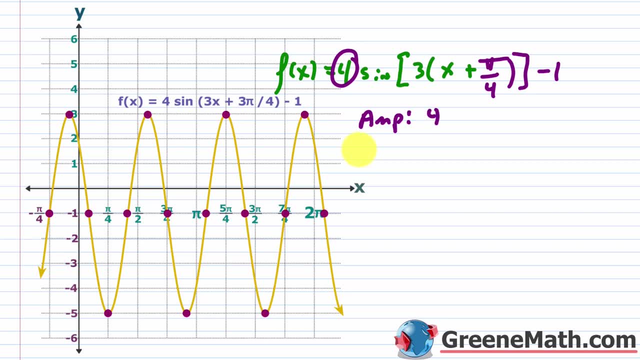 and the minimum. So we would know it would be 4 and negative 4.. So the range here is going to change because of this minus 1.. Instead of 4 and negative 4, what you're going to have is everything shifted down by a unit. 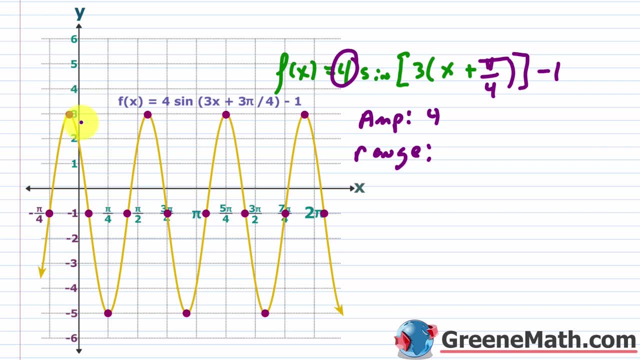 So now, instead of 4 for the maximum y value, you're going to have 3.. Instead of negative 4 for the minimum y value, you're going to have negative 5.. So your range is going to be from negative 5 to positive 3.. 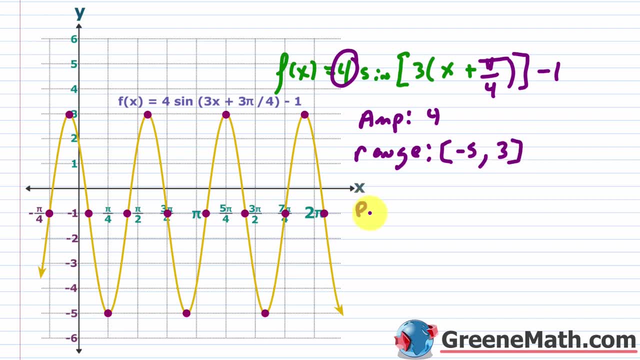 So keep that in mind Now when you talk about your period. your period that's going to be 2 pi over b and b is just 3.. That's pretty easy, And then you're also going to need the quarter periods. 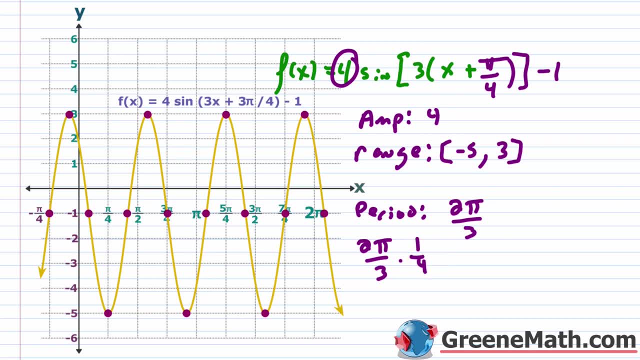 So 2 pi over 3 times the 4th. Let's go ahead and cancel this 2 with this 4 and get a 2.. So your quarter periods here are going to be pi over 6.. So I'm going to put quarter: quarter period is just going to be pi over 6, okay. 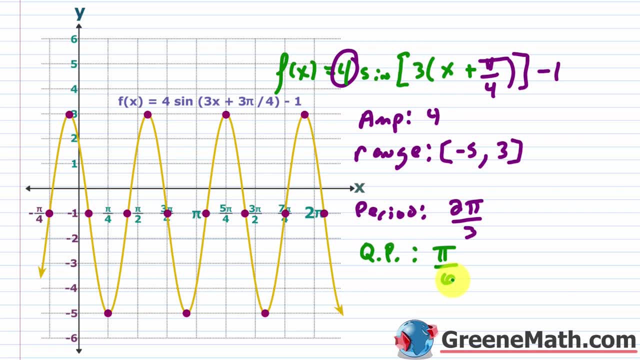 So let's talk about how we can get this graph. if you're trying to do this quickly, Remember you start off with 0 comma 0 on the basic sine graph, So think about all the things that are going to be done. You're going to have a phase shift of pi over 4 units to the left. 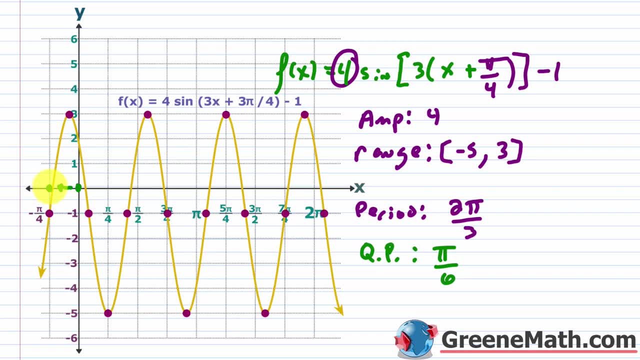 So that's going to take me this way: by pi over 4 units. So that point would be here now And then we're shifting down by 1 unit, so that point's going to be right there, okay, So I got moved from 0 comma 0 to that point, which is going to be negative pi over 4, comma. 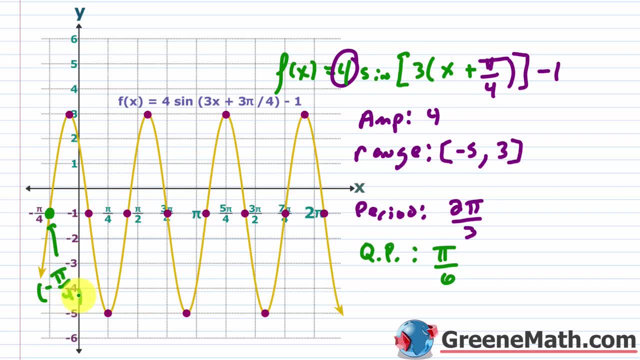 the y value instead of it being 0,. right, normally that's the x-intercept. it's been shifted down by a unit, so this is going to be negative 1, okay Now as we go to the next x value. so you've got this one, which is at the quarter. this: 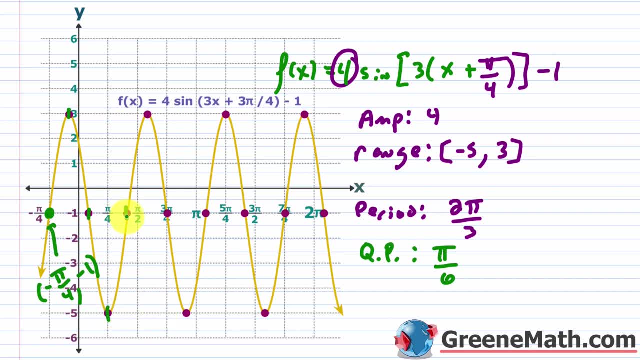 one which is at the half, this one at the 3 quarter and this one at the full period. we're just adding quarter periods, right? So we're adding pi over 6 to get to the next x value, okay, So when I add pi over 6 to negative pi over 4,, I'm going to get negative pi over 12, okay. 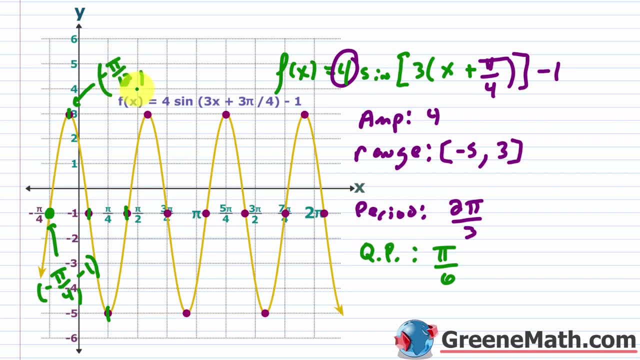 So this is negative pi over 12.. How do I get my y value? Again? this is positive here. so I know at a quarter way through I'm at the maximum and the maximum is going to be 3, okay, So pretty easy there. 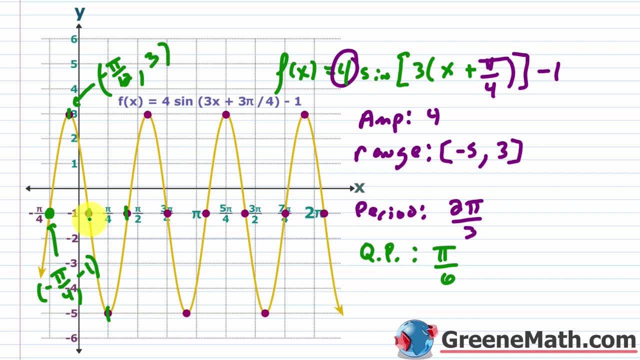 Then, as I go back, this would have been an x-intercept right, But it's not. it's been shifted down by one unit, so I know the y value here is going to be negative 1, that's pretty obvious. 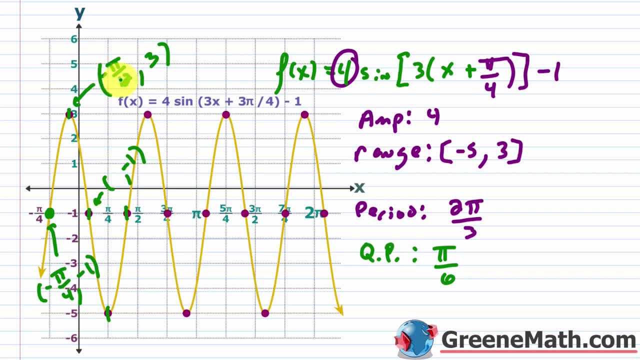 And then for the x value, I just take my negative pi over 12, and again I'm just going to add my pi over 6,, just add a quarter period, and that's going to put me at pi over 12.. So this one is pi over 12,. right there, okay. 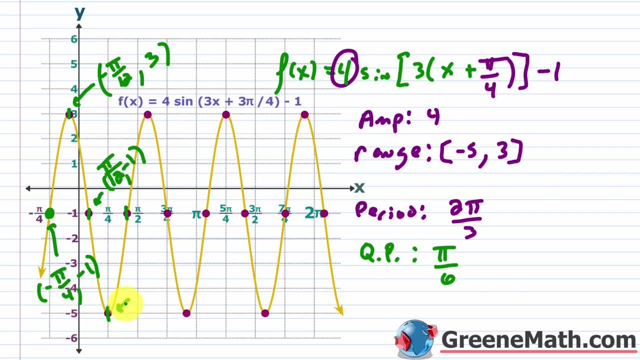 And then at 3 quarters of the period, I know I'm going to be at my minimum right, and the minimum is negative 5.. Negative 5 in there, okay. And for this guy I just take my pi over 12, and I add another quarter period, so pi over. 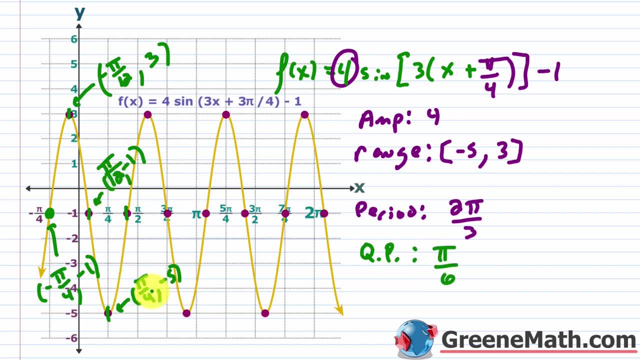 6, and that's going to give me this pi over 4.. So this is pi over 4, comma negative 5.. Then to get my last point here in this cycle, what I would want to do is add pi over 4,. 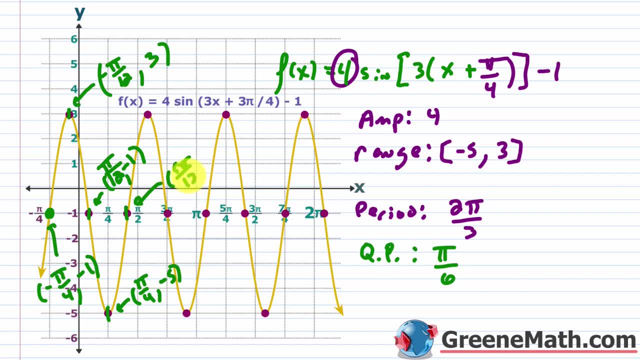 and pi over 6, that's going to give me 5 pi over 12, and I know the y value. that would have been an x-intercept. it's been shifted down by a unit, so instead of 0, it's going. 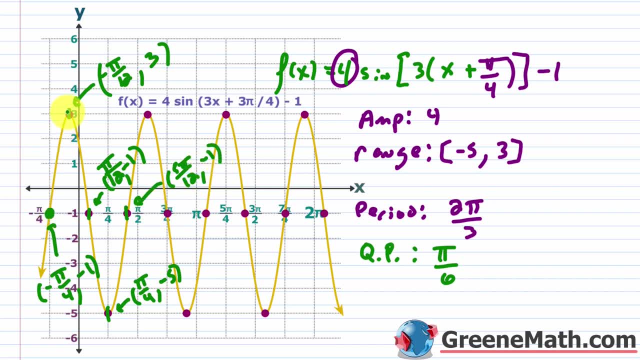 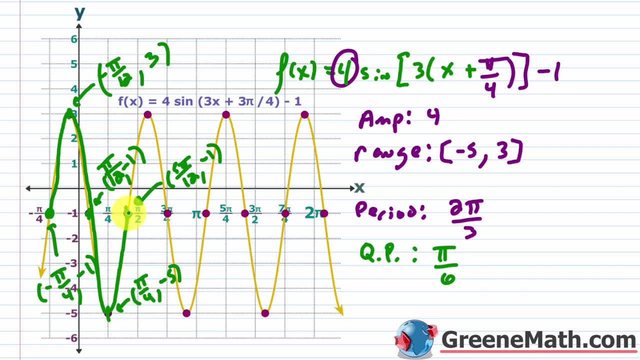 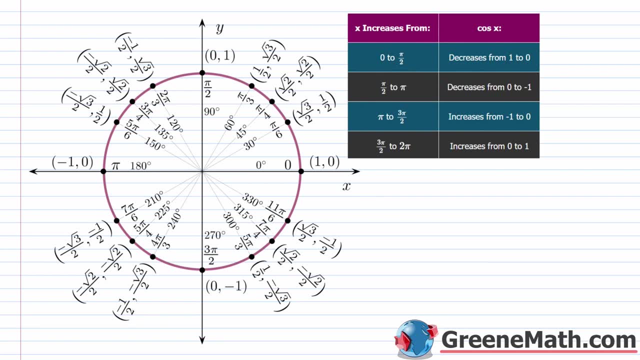 Just connect these guys with a smooth sine wave and you're basically good to go. If you want to go to the right or to the left, you're just making repetitions of that one cycle. All right, now that we've mastered graphing the sine function, we're going to move on. 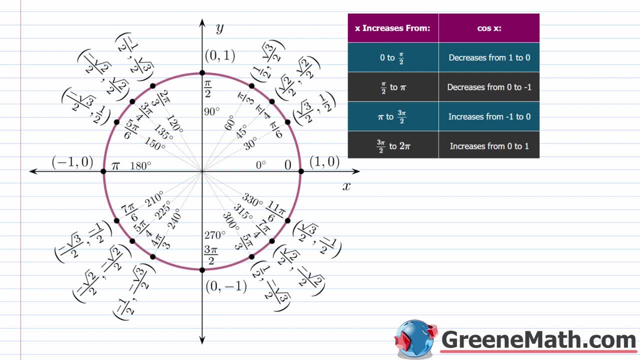 now and talk about graphing the cosine function. So the reason I spent all of the lessons so far on the sine function: it's a little bit easier to start with 1. Take one function, learn all of the graphing transformations and then take that knowledge. 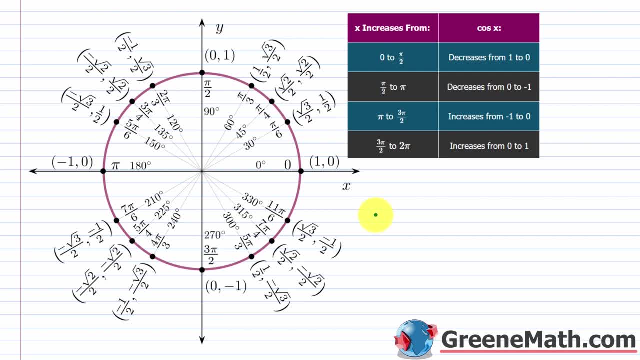 and apply it to the other one. okay, It's the same process. So if I think about, f of x is equal to the cosine of x, how will this graph be different from f of x equals the sine of x. Well, basically, you take your sine graph and you do a phase shift of pi over 2 units. 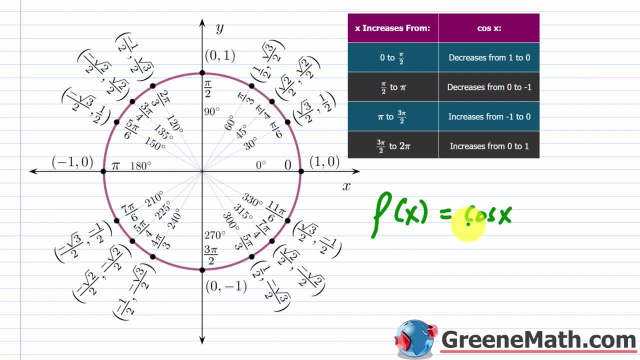 to the left, and you're going to have your cosine graph. You'll see that in a moment. So all we really need to think about is how this guy is going to move. Okay, so let's do a graph. Let's do a graph. 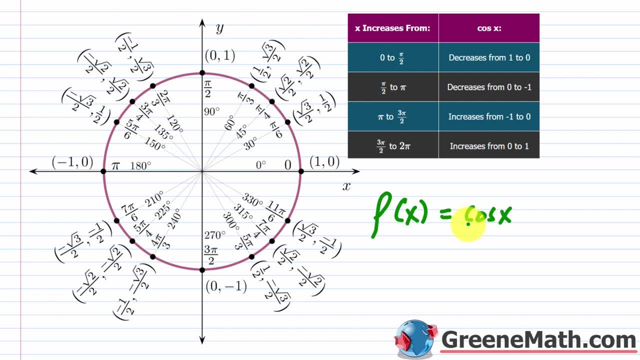 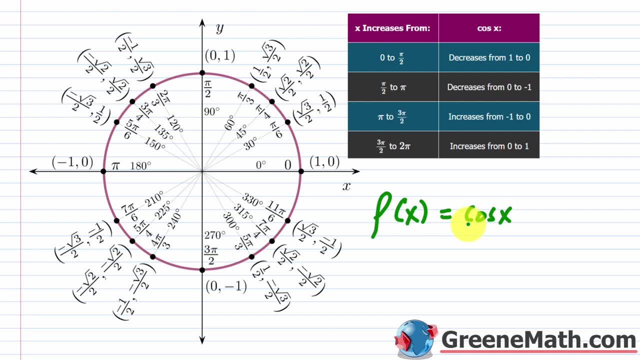 there. How is that going to be different Once you memorize that? you just take the knowledge from the sine graph, that you learn those strategies, those techniques and you apply it to the cosine graph and you're good to go. So I'm just going to think about these. 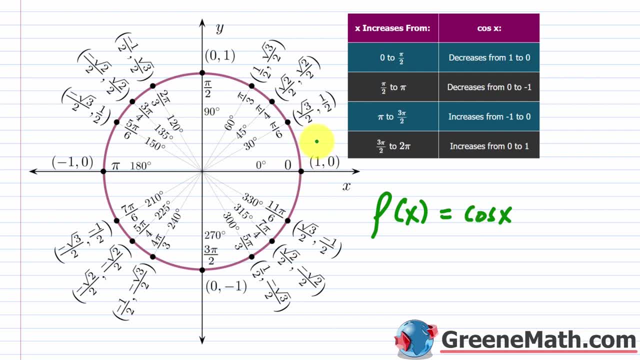 quadrantal angles We start with an x value of zero would produce a cosine value or a y value of one, okay, And then as we go to pi over two, we're decreasing, right. So we're going to end up at zero when our x value or angle is pi over two. Then, as we continue to pi, we're decreasing. 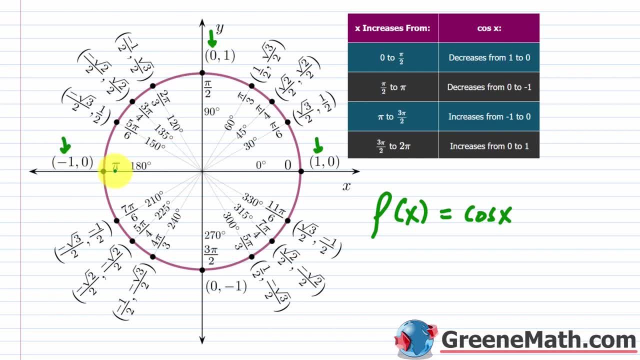 from zero down to negative one, okay. And then, as we go from pi to three pi over two, we are increasing from negative one up to zero, okay, So right there. And then, lastly, as we go from three pi over two to our two pi- right, We're making one full rotation- We are increasing from zero. 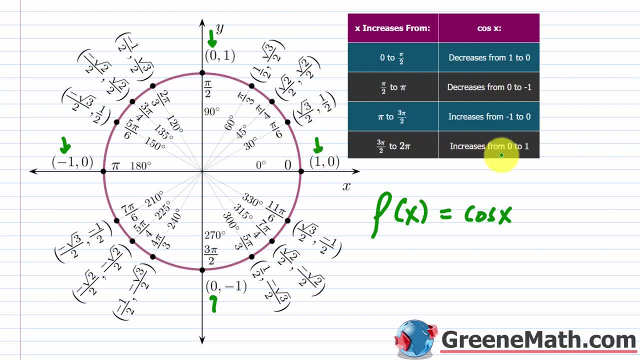 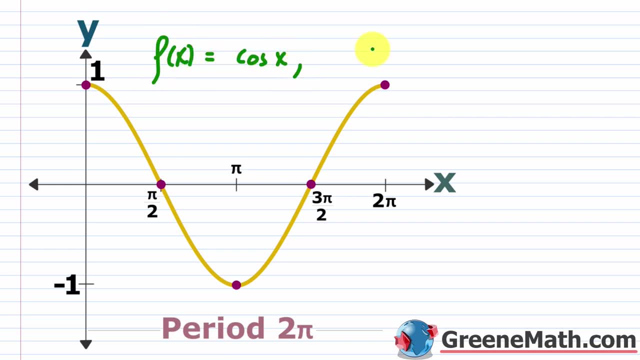 to one. okay, So you can refer to this table if you want to have some notes on that. Now, when we think about this guy over one period. so f of x is equal to- I'm going to put cosine of x. I'll say that zero is less than. 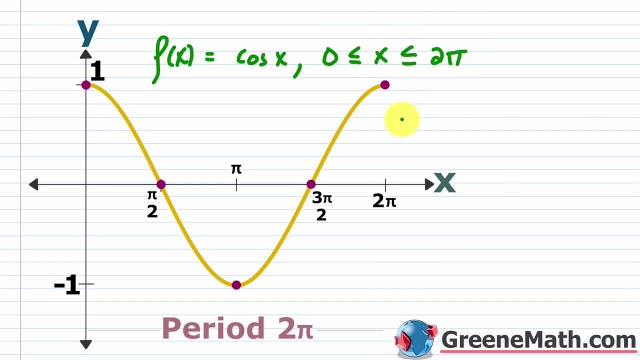 or equal to x, which is less than or equal to two pi. So this is just one period. You want to think about how these points are going to be different from the sine graph. If you memorize those differences, you're basically good to go. Your period here is the same. It's still going to be. 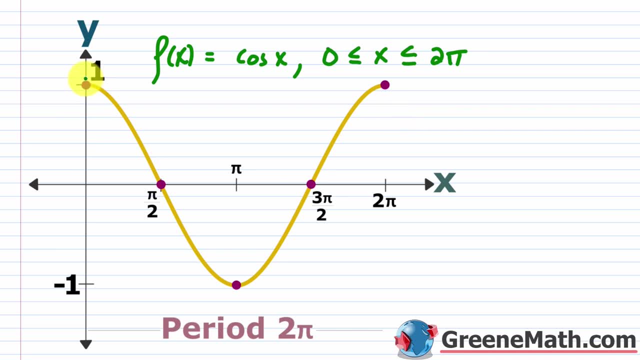 two pi. We should know that from the unit circle. Now you'll notice that you have a maximum here and a maximum here, And this if I draw a line down the middle. I want you to notice that you could take this point and reflect it across this line. 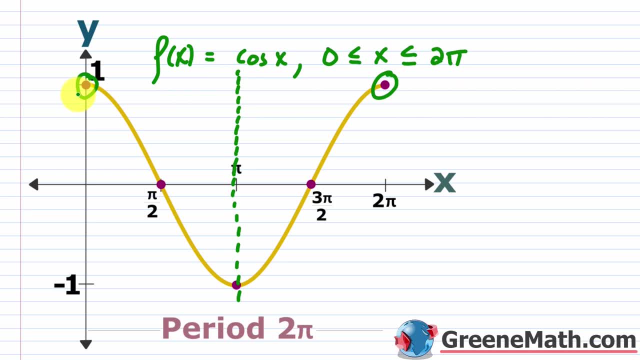 and you'd end up with this point. Remember that is an even function, right? So where f of negative x is equal to f of x, We've seen this with the squaring function, right? If you saw something like f of x equals x squared. it doesn't matter if I plug in a two there. two squared is. 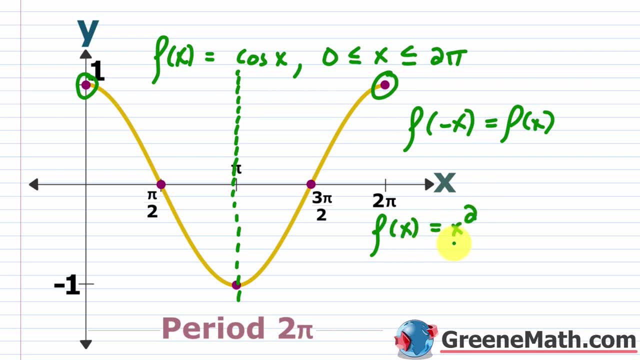 four, or a negative two. negative two squared is also four. You get the same y value. okay, So cosine is going to be an even function. We'll talk more about that in a moment. Okay, So another thing you'll want to think about- and this is going to be an even function- is that you're going to 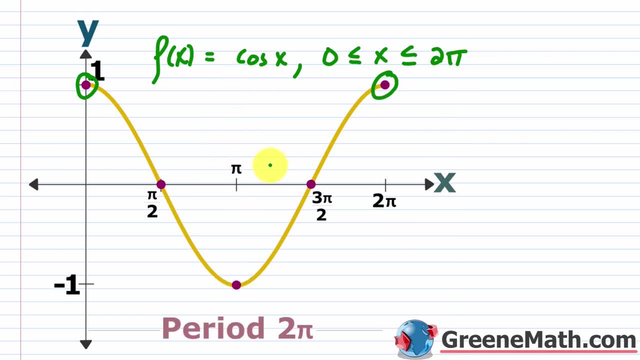 have a cosine of x and you're going to have a cosine of x and you're going to have a cosine of x. you'll want to think about is the fact that with the sine graph, remember, you had three x intercepts. You had an x intercept at the beginning, the middle and the end. okay, Here you only have. 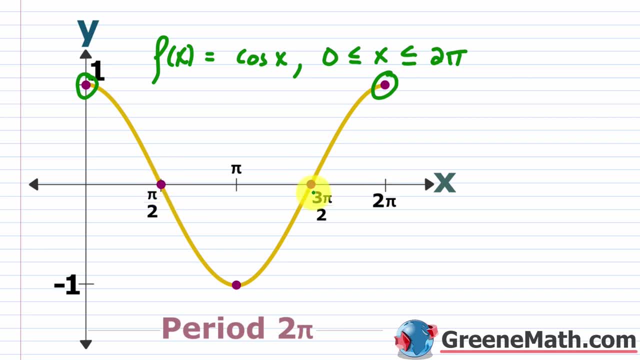 two x intercepts and it's going to be at the quarter of a period and three quarters of a period, okay. And then your minimum occurs at halfway, okay. So you want to remember that you start at the maximum, you end at the maximum halfway through. you're at the minimum, okay, And a quarter. 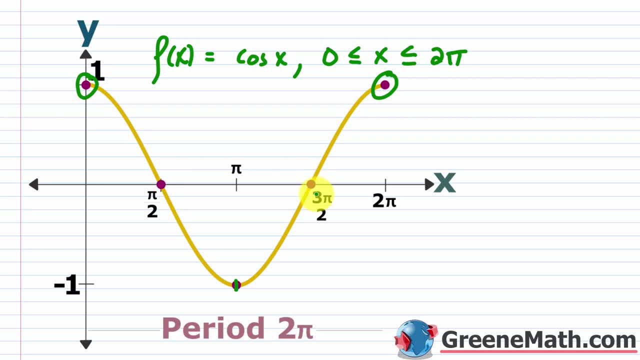 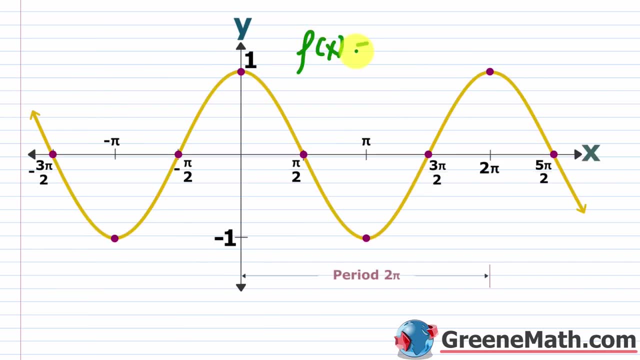 way through, and three quarters way through, you're at the x intercept. That's really all you need to memorize. You just take the other information from the sine graph and you're good to go. Now let's extend this to the left and right. So this is: f of x equals the cosine of x. So here's going. 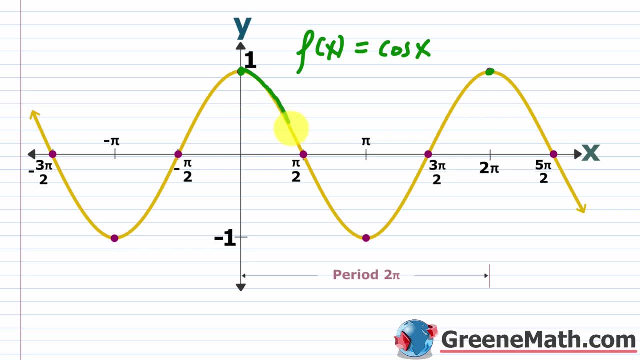 to be one period from here to here. okay, So one period Again. this is just the sine graph that's been phase shifted to the left by pi over two units. okay, That's all it really is. It's the same type of graph. Now a couple of key things. this f of x equals the cosine of x. it's continuous. 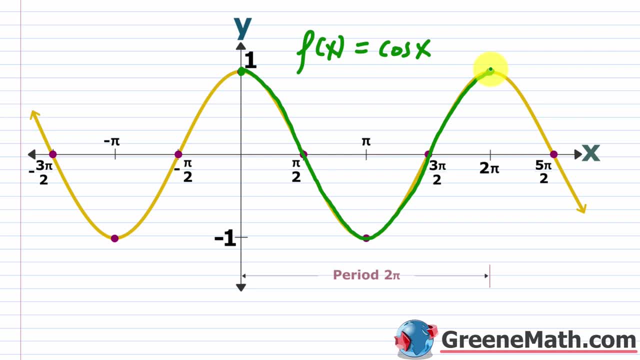 across this entire domain. So, just like the cosine of x, it's continuous across this entire domain. Again, the domain for each is going to be all real numbers. The period for each is going to be two pi, So that stuff's the same. The range is negative one to positive one. That's the same, The x. 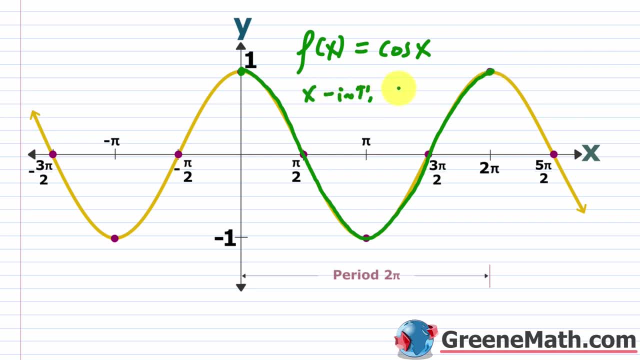 intercepts. this is going to be different. So the x intercepts is going to be of the form you're going to have two n plus one times pi over two. okay, I should probably move this so it's a little bit more clean. Let me move this down there And basically n is any integer. Let me make that a. 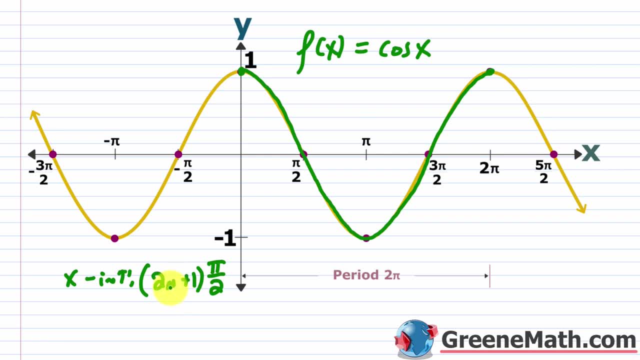 little bit better because that's a little bit more clear. So let's move this down there And that's bad in terms of handwriting. Let's say n was zero. Two times zero is zero, So you'd have one times pi over two. So that's this x intercept here. okay, If you put in a one, you'd have two. 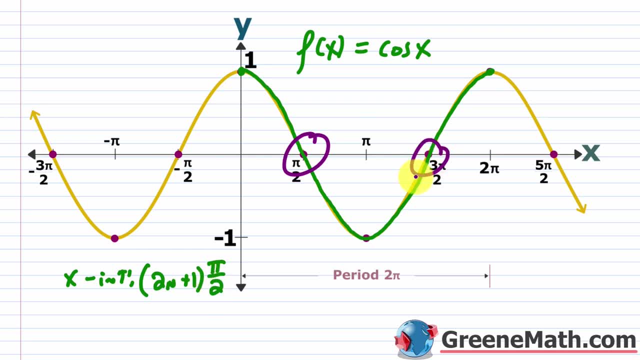 plus one is three. Three times pi over two is three, pi over two, so on and so forth. Now the last thing I want to do is talk about the fact that this guy is an even function. We already saw that right when I basically drew a vertical line at x equals pi, But you should know that basically. 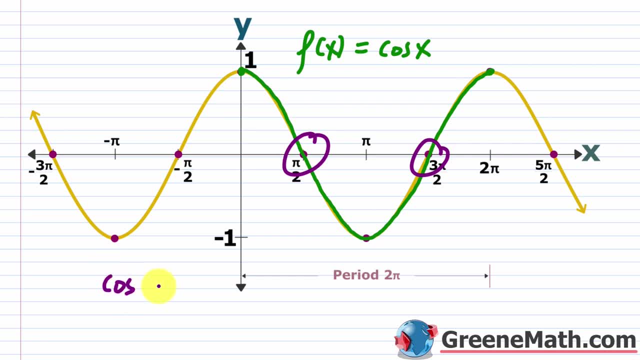 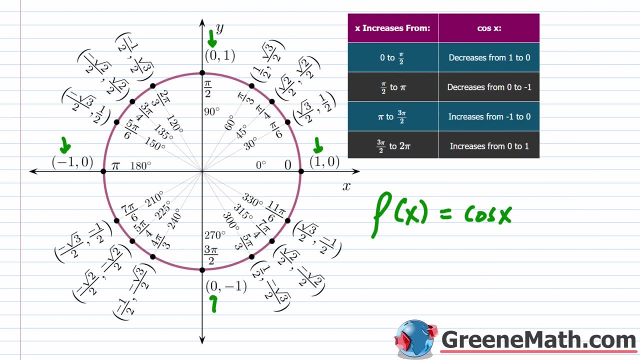 with cosine of x. you could say, oh, this is an even function. So you could say, oh, this is an even function. Let's say that the cosine of negative x is equal to the cosine of x. We can go back to the unit circle and you can grab a value real quick. Let's say you grab pi over six and 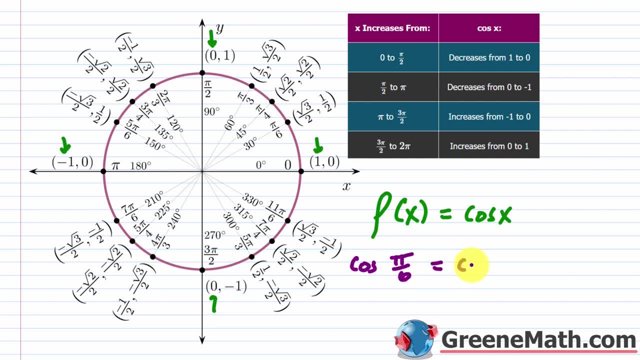 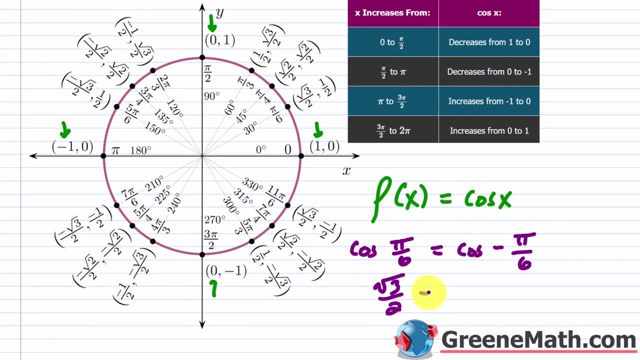 you can say: the cosine of pi over six is equal to the cosine of negative pi over six. Really easy to prove that Cosine of pi over six is square root of three over two And the cosine of negative pi over six. I'm just rotating clockwise now, So I'm coterminal with 11 pi over six. So this: 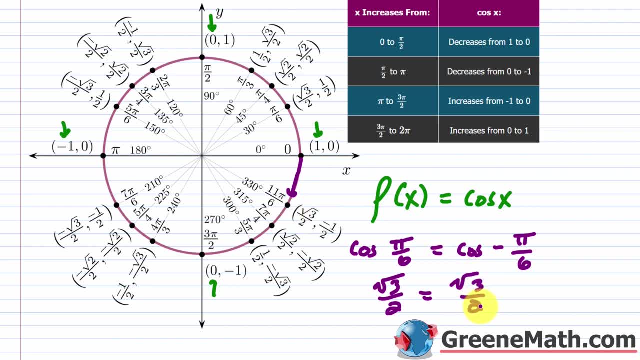 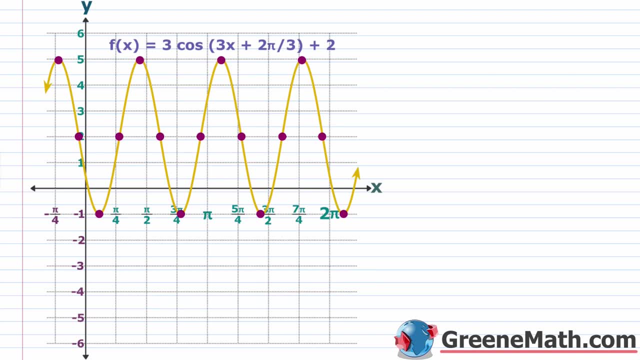 would be square root of three over two as well. okay, So cosine is an even function. Okay, let's take a look at one example with graphing cosine. I'm going to put all the different transformations into this guy. Again, if you can do this for sine, you can already do it for cosine Now. 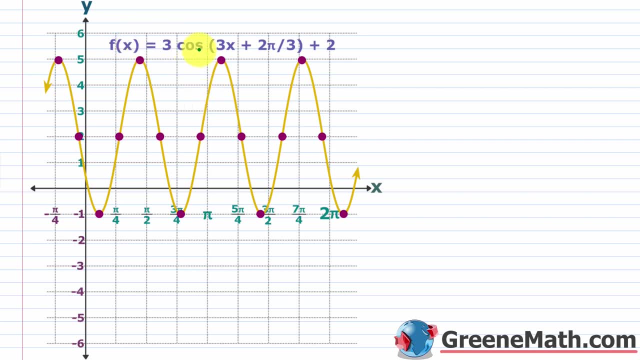 what I'm going to do is rewrite this. to start, You have: f of x equals three times the cosine of three, x plus two, pi over three. Then you have this plus two. So let me write: f of x is equal to: I've got three times the cosine. 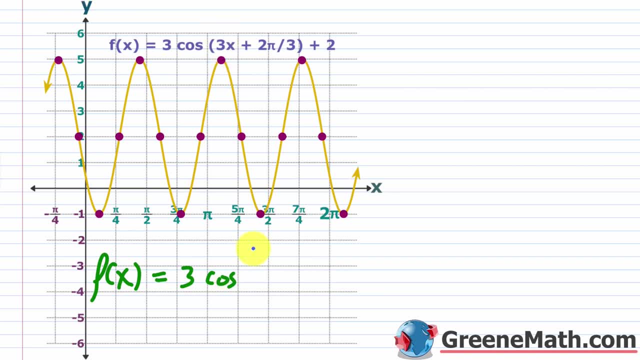 cosine of. I'm going to go ahead and factor this three out Again. I think this is the simplest way to identify the phase shift, but you don't need it, So it's up to you. So three times, inside the parentheses, divide everything by three. Three x divided by three is x. Then plus, if I had two pi. 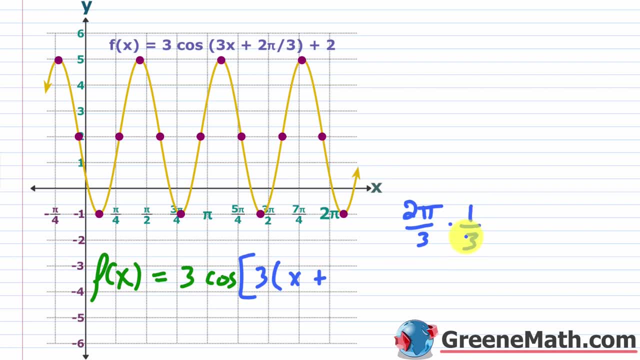 over three. and I multiplied by a third- same thing as dividing by three- this would be two pi over nine. Okay, close that down. And then don't forget your plus two at the end. Okay. so now that we know that this three out in front the absolute value of that guy, which is just three. 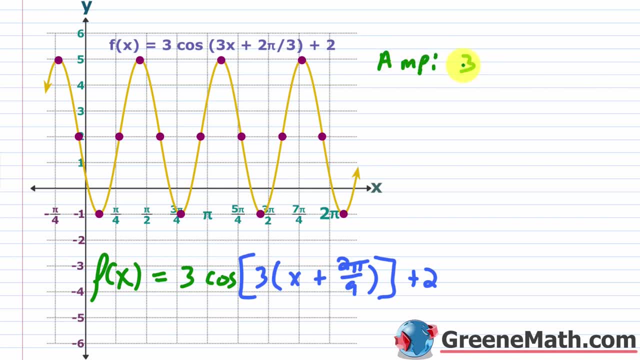 is the amplitude. Okay, so that's going to be three. Now, with the normal cosine graph, just like a normal sine graph, it's going to tell you your minimum is at negative three and your maximum is at positive three. But if you look at the graph, that's already drawn. 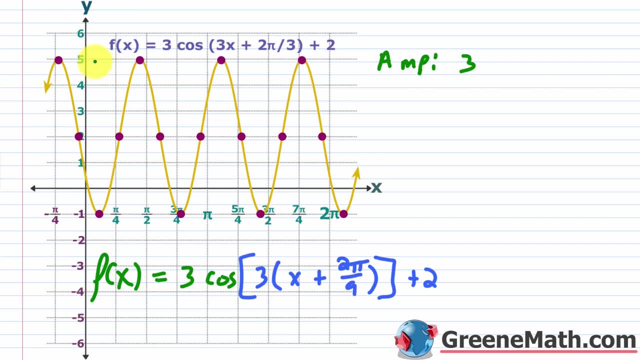 you see, the minimum is at negative one and the maximum is at five. So what's going on? You have this plus two at the end, okay, and that's giving you a vertical shift up. So, instead of negative three for the minimum. 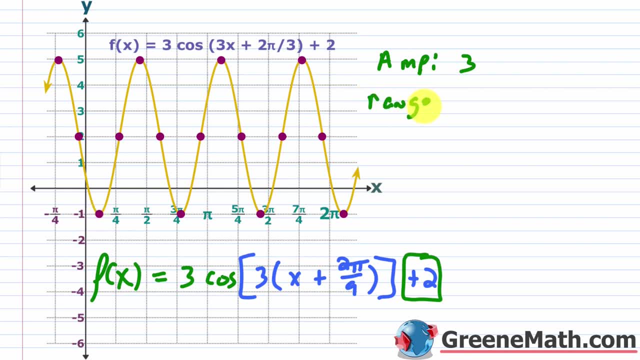 two units and you get to negative one. So if I think about my range, okay, the minimum is now going to be negative one. The maximum again, it would have been three add two units. now it's going to be five. Okay, and we're going to use this in a little while when we start getting these. 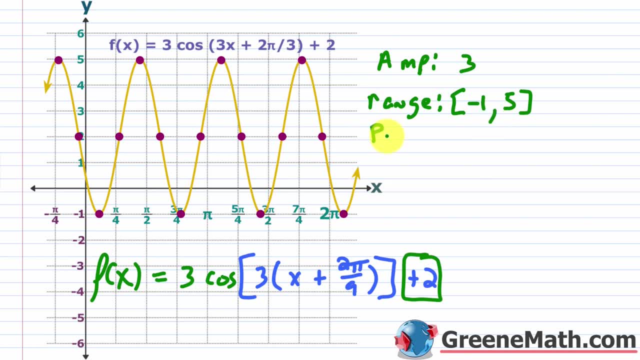 points Now. additionally, when I think about the period, it's going to be two pi divided by b. Now b here is three, so just two pi over three. If you want the quarter periods again, this is for us to. 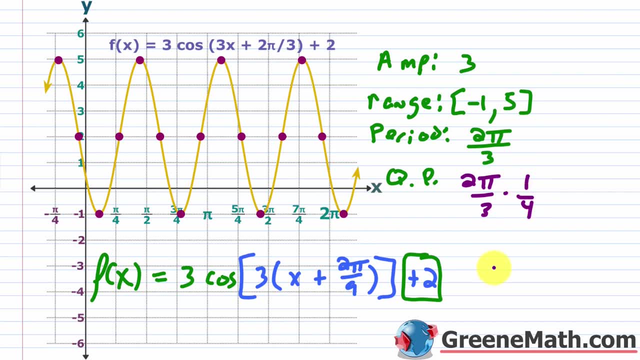 Well, it's just two pi over three multiplied by a fourth. So basically this cancels with this and gives you a two. So this is pi over six. Okay, so we're going to have pi over six for the quarter periods. And then when we think about the phase shift, so let me put the phase shift in here. 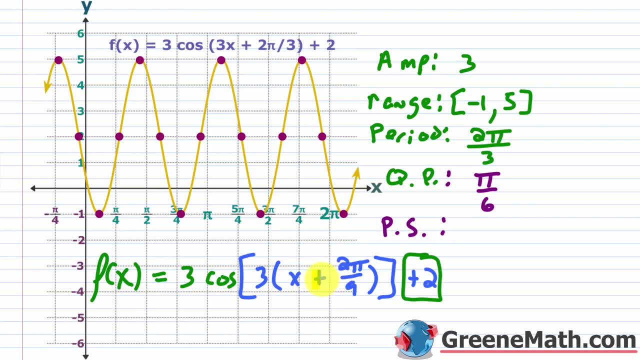 you have x plus two pi over nine. So again, if you have plus two pi over nine, I'm shifting to the left by two pi over nine units. So that means I'm going to shift to the left by two pi over nine. 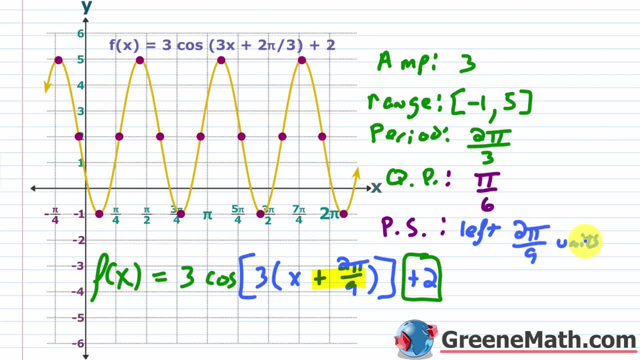 units. Now, the last thing I want to put in here- and I'm running out of room, so let me just put it off to the side- my vertical shift, as we talked about earlier. I have a plus two here, So that's. 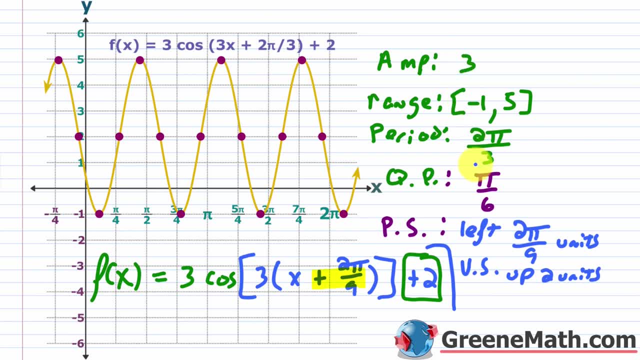 up two units. Okay, So now that we've identified all these things from just looking at our function, we can go through and think about how our points would have moved based on the original cosine graph. So it's really, really easy, Okay, Now what I would say is that this guy, based on the 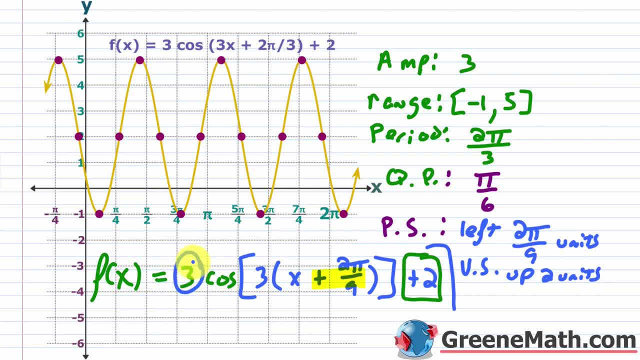 has been stretched vertically by a factor of three from that guy. It's been compressed horizontally by a factor of one over three. It's always one over B, B is three. So it's been compressed horizontally by a factor of one third. And then we've had a phase shift of two pi over nine units. 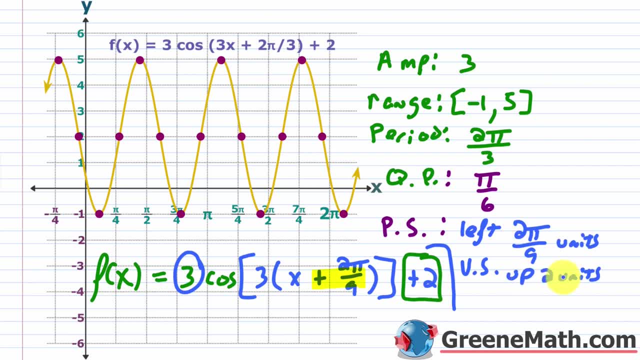 left and a vertical shift up by two units. Okay, So that's all our different transformations. So if we go to our original cosine graph, remember the cycle starts at the maximum. The x value is zero and the y value is one. Okay, So, based on this function here I know I'm going to start at the maximum. The maximum is: 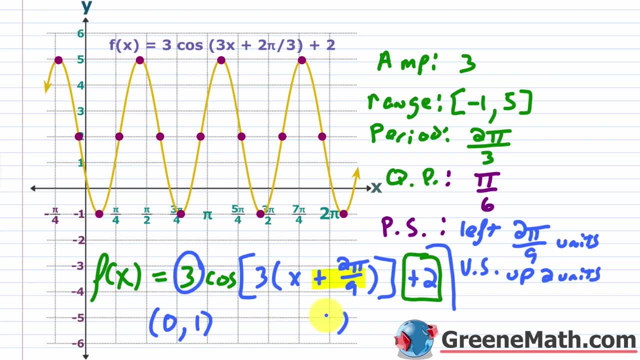 five. So I know the y value for this first point is going to be five. What's the x value going to be? Well, I'm just going to consider this phase shift, which is two pi over nine units left. So two pi over nine units left. So that would give me a negative two pi over nine. Okay, And 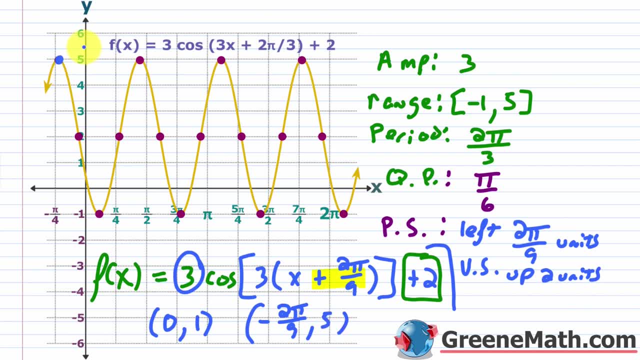 then comma five. So that's going to be this point right up here. Okay, That's going to be the first negative. Let me put my two pi over nine comma five. Okay, So pretty easy to get that point. Now, when you go to get the other points, what I would suggest is just getting your y values first. 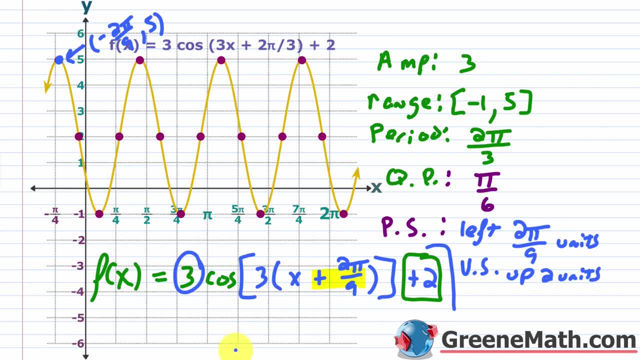 They're really easy to figure out. Remember, at the beginning of the period and at the end of the period you're at the maximum. So here's your beginning and here's your end. Okay, So you're going to be at the maximum. So let me put a comma here and then put a five. Okay, So I know the y. 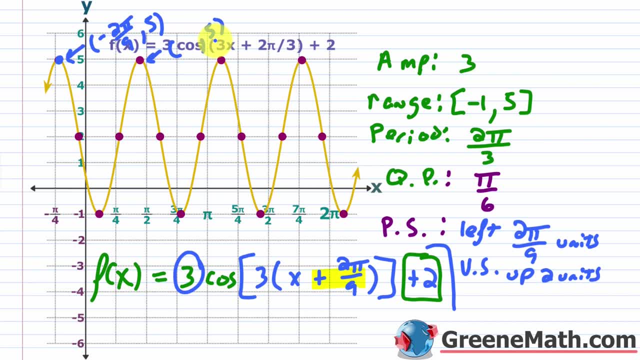 value. there is five. I know that halfway through I'm at the minimum. The minimum is negative one. We already figured that out, So that's going to be right here. Let me put a comma and then negative one At a quarter way. 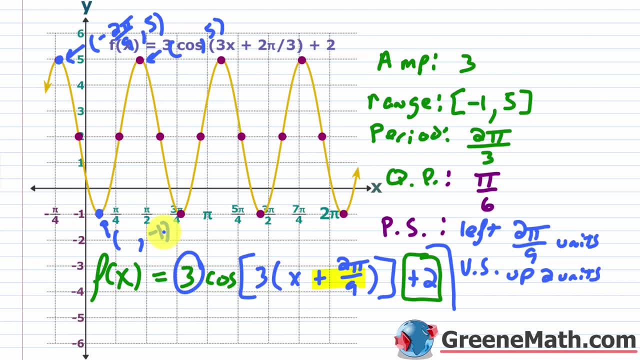 through the period and three quarters way through the period, you would have had an x intercept. But because we have this plus two or this vertical shift up by two units, now the y coordinate is going to be two. Okay, So for right here the y coordinate is going to be two, And 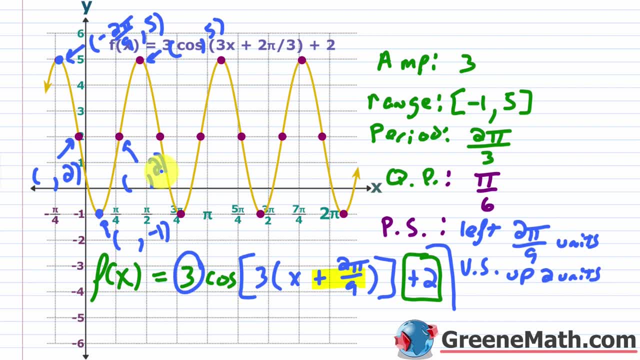 for right here the y coordinate is going to be two. Again, if you find this confusing what I'm doing, you can always take your x values, plug them into the function and evaluate, and you can get your y values that way. This is just quicker for me and for most people. as they sketch the 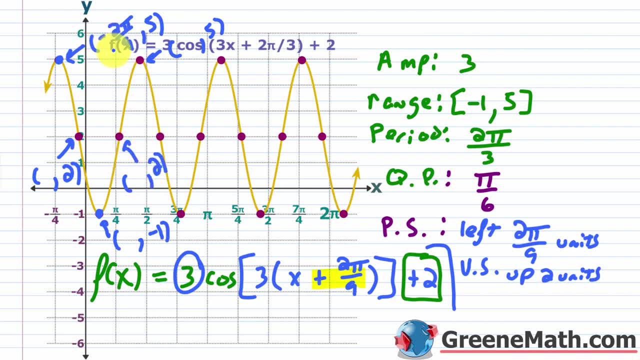 graph. Now to get these four missing x values. you already have the first one, You're just going to add quarter periods. Okay, So I'm going to add pi over six to the existing x value. So negative two pi over nine plus pi over six is going to give me negative pi over 18.. So negative pi over 18.. 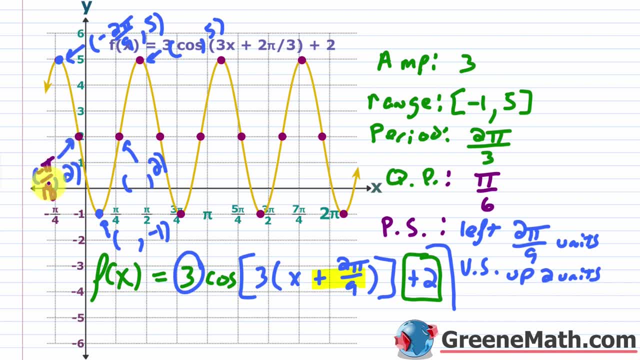 Okay, So that's going to be the x value for this point right here. Okay, So negative pi over 18, two. Then, as I get to my minimum, I add another pi over 6 to this negative pi over 18, and what I'm going to get is pi over 9.. So this point would be: 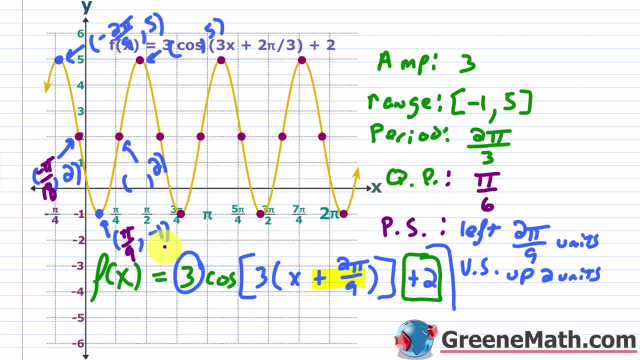 pi over 9 comma negative: 1.. Then I add another pi over 6 to this pi over 9, and I'm going to get to 5 pi over 18.. So 5 pi over 18 comma 2.. And then, lastly, I add another pi over 6 and I'm going to 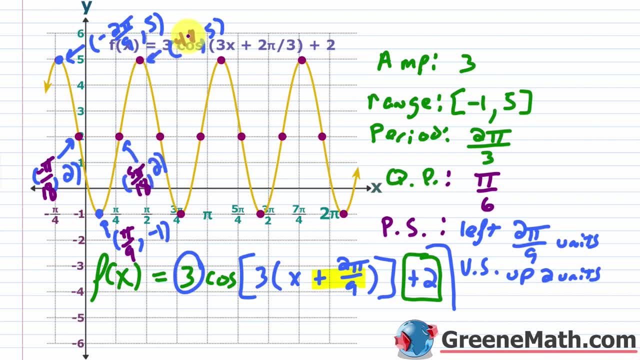 get to the x value for this point, which is going to be 4 pi over 9.. Let me make that a little bit better. Okay, let me make that a little bit better. So 4 pi over 9 comma 5.. Okay, so this would be. 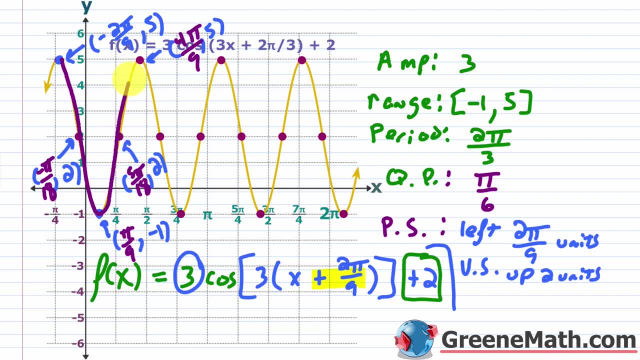 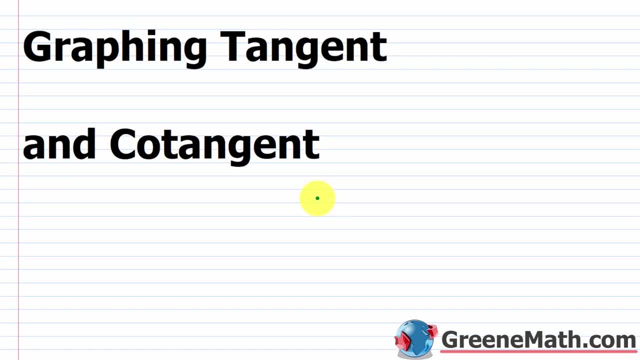 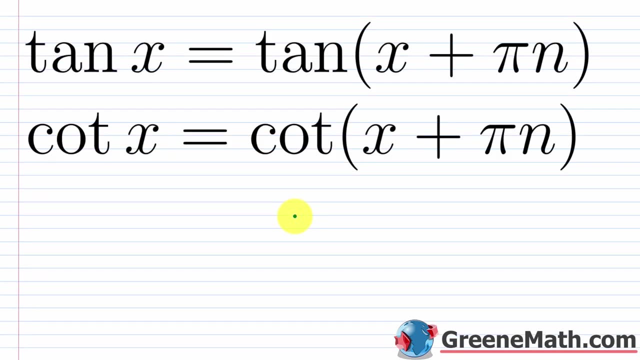 one cycle, okay, for our graph. And again, if you want to keep going to the left or the right, you're just making repetitions of that one cycle. In this lesson we're going to talk about graphing tangent and cotangent, All right. so in the last lesson we talked about how to sketch the graphs for 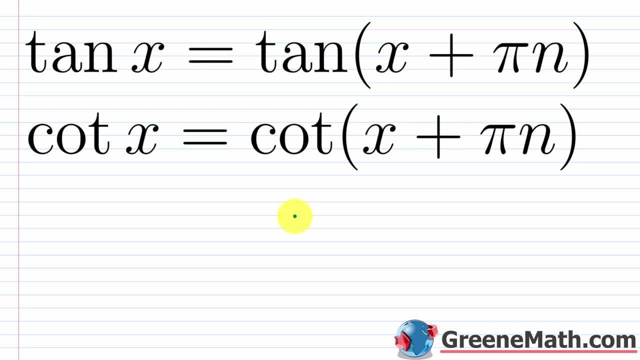 sine and cosine, and we found that the process is really not that bad. The main thing to understand when you're in this section is that you are not expected to make a perfect graph. You're just expected to know the key information And how you could sketch the graph if you had to. Generally speaking, we're always going to use 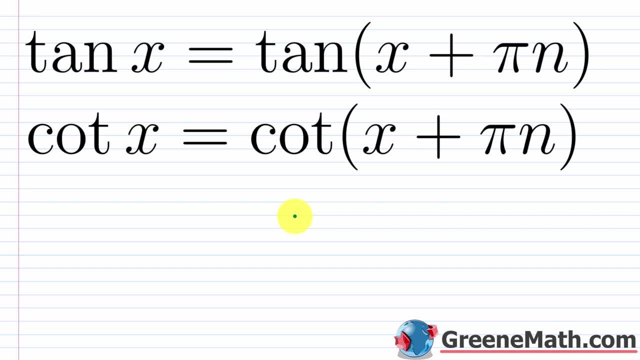 computer software, either something that's online or a graphing calculator like a TI-83, to sketch our graphs. So, with that being said, let's go through how to sketch the graph for tangent and cotangent. We're going to start with a different period, So basically we know that the period 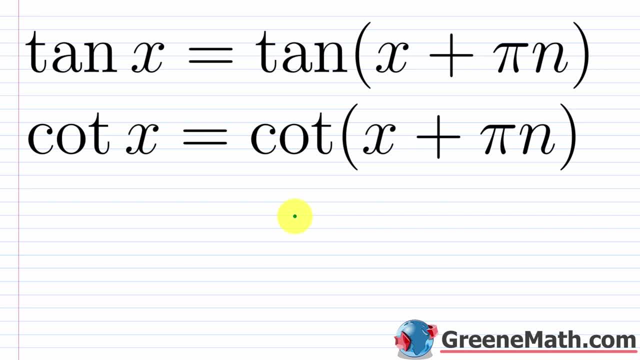 for sine and cosine is 2 pi. But when you work with tangent and cotangent you need to know that that's extremely important, especially when we get to solving trigonometric equations. So something like the tangent of x is going to be equal to the tangent of x plus pi, n, where n is any integer and 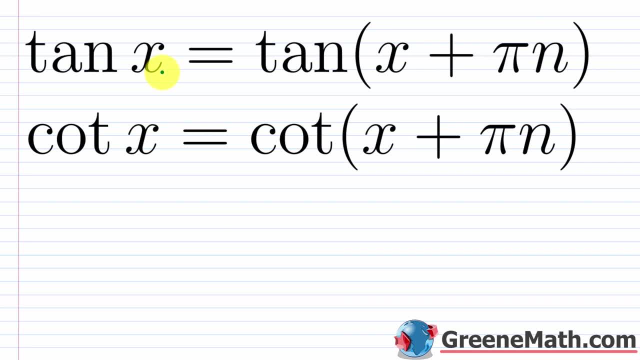 we would also say that x is a member of the domain. Remember that when you work with tangent you have places where it's undefined. Then we have: cotangent of x is equal to the cotangent of this x plus pi, n, again where n is any integer and x is a member of the domain. So let me just quickly demonstrate. 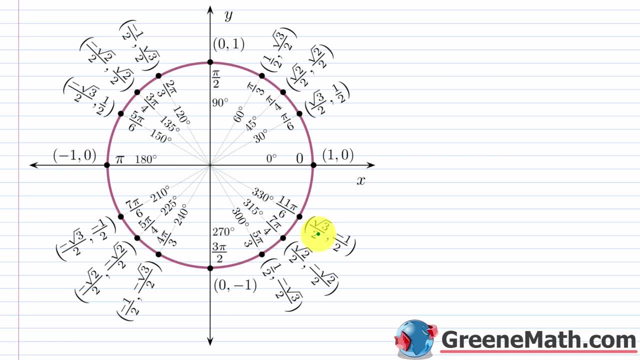 that the period for tangent and cotangent is equal to the cotangent of x plus pi, n, where n is any integer and also cotangent is going to be pi. You can show this with identities, but we haven't gotten that far yet. First off, I'm just going to pick something like pi over 6 for the angle. 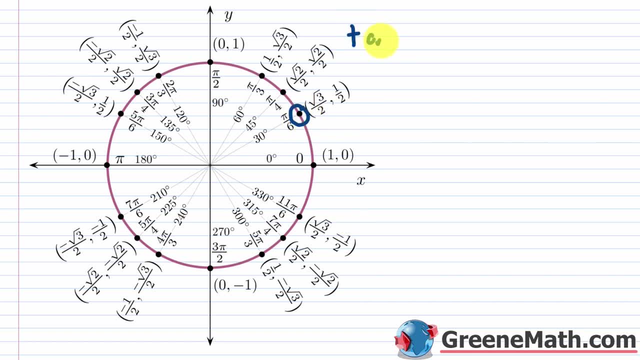 So this guy right there, And you know that if you want the tangent of pi over 6, you can find it as the sine of pi over 6 divided by the cosine of pi over 6.. In other words, we should know that the tangent of x is equal to your sine of x over your cosine of x. 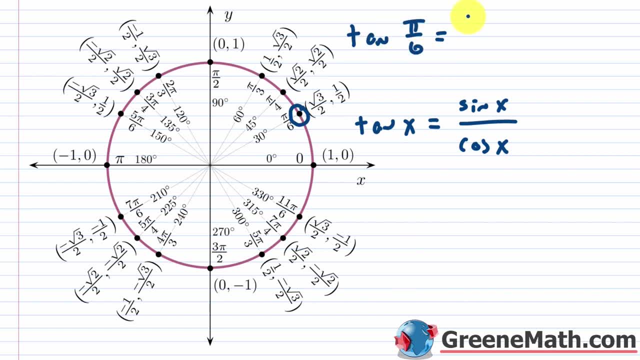 So the tangent of pi over 6 is going to be equal to the sine of pi over 6, and then this would be divided by the cosine of pi over 6.. So what would this be equal to? We know that the sine of pi over 6, again, that's going to be given by the y coordinate right there. so that's. 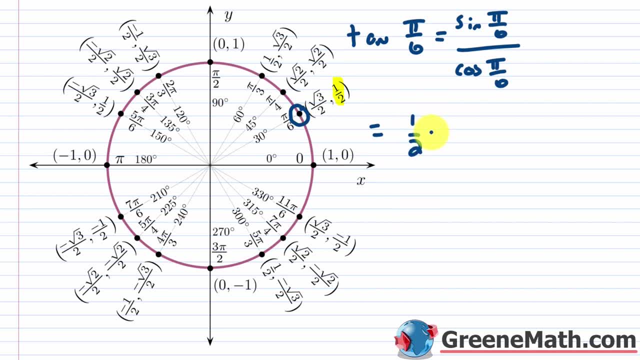 one half. So let's write that. How do we divide fractions? We multiply by the reciprocal. So this is times. You would have the cosine of pi over 6, that's square root of 3 over 2, but you're going to find the reciprocal of that. So this is going to be times 2 over the square root of pi over 6.. 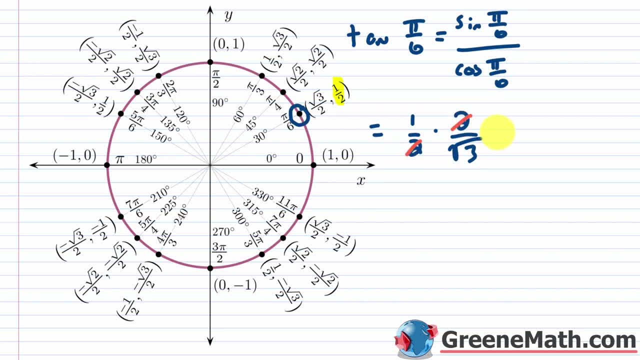 And then basically the 2's are going to cancel. And let's say that this is 1 over the square root of 3.. We want to rationalize the denominator here, So times the square root of 3 over the square root of 3.. So this equals the square root of 3 over 3.. So this is the square root of 3 over. 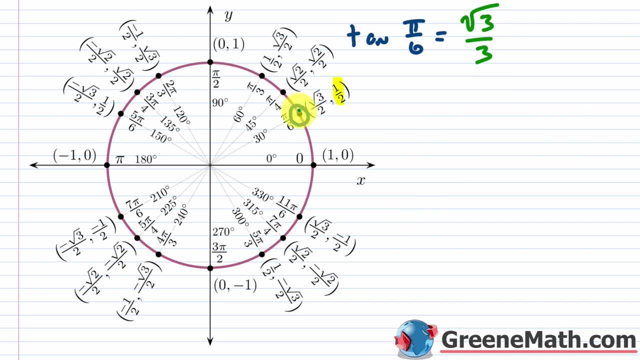 3.. Now I want you to notice that if you add pi, or you could say if you rotate by pi. So I'm going to come over here into quadrant 3 and we're going to be at 7 pi over 6.. Now I want you to notice that if you add pi over 6, you're going to get the square root of 3 over 3.. 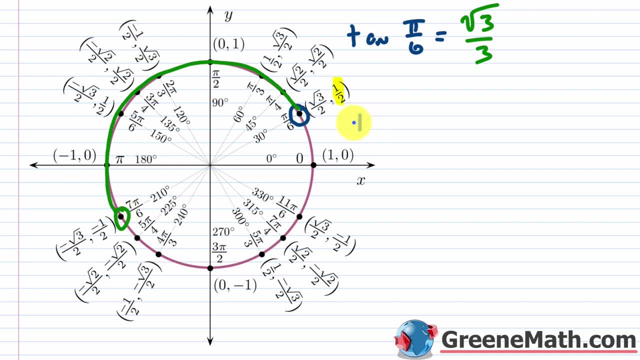 Now I want you to think about if I found the tangent, So the tangent of 7 pi over 6.. What would I get? Well, you're going to find that you're going to get that same square root of 3 over 3.. 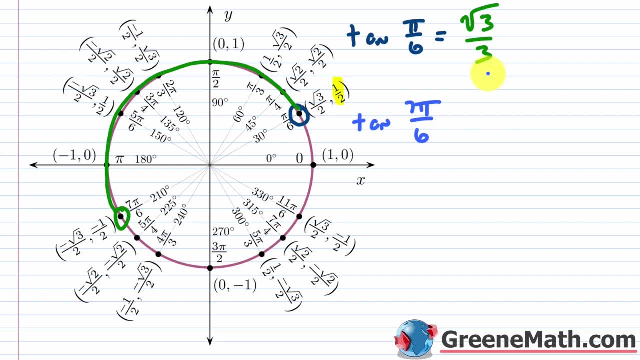 And the reason for that is you're dividing, in terms of absolute values, the same numbers. It's just that now you're going to be dividing a negative by a negative, which is also going to give you a positive. So, in other words, this is going to turn into your sine: value is negative. 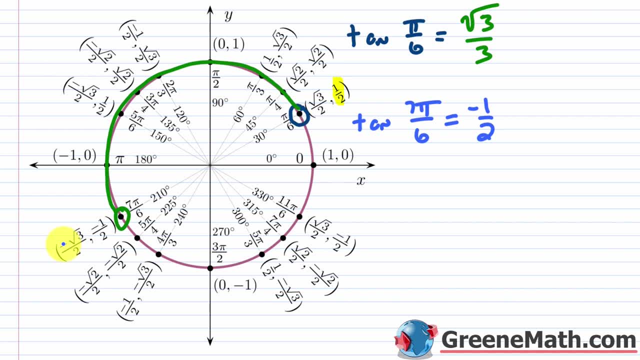 one half and then divided by your cosine value, is negative one half. So you're going to get the cosine value, which is negative, square root of 3 over 2.. We're going to again multiply by the reciprocal, So let's go negative. We're going to go 2 over the square root of 3.. And so the negative. 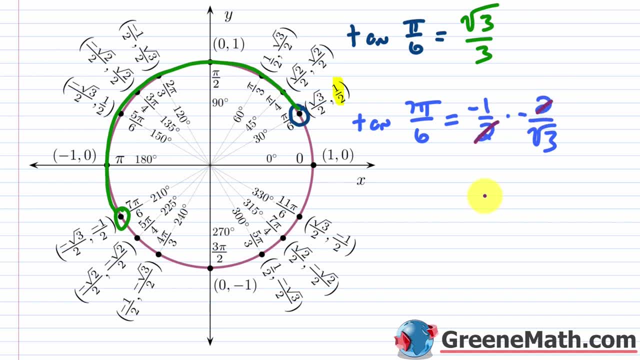 times, the negative will give you a positive, The 2's will cancel. So this would end up being 1 over the square root of 3, which we know. if we rationalize the denominator, that's going to be the square root of 3 over 3.. So you can see that the tangent of pi over 6 and the tangent of 7 pi. 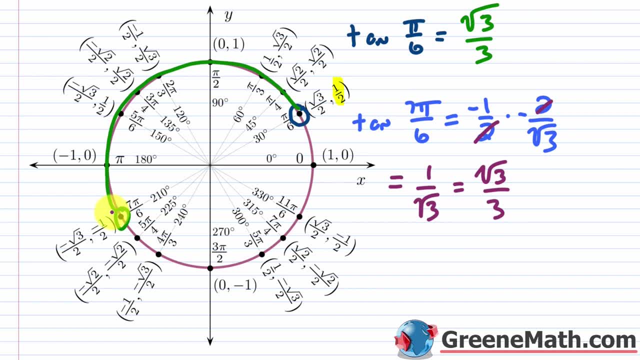 over 6. that's the same. So that's one way you can demonstrate this. I'll show you with some of the other ones So you can see the stuff in quadrant 2 and 4.. So that's where tangent is negative. So 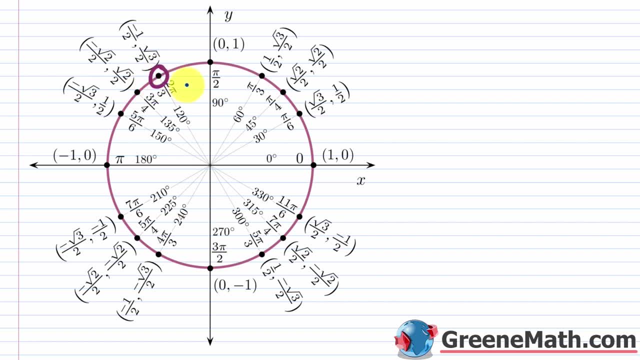 let's say, you pick something like, let's say, 2 pi over 3. So that guy right there And that color doesn't show up so well. So let me do that like that. And again, if you add pi to this, So if you, 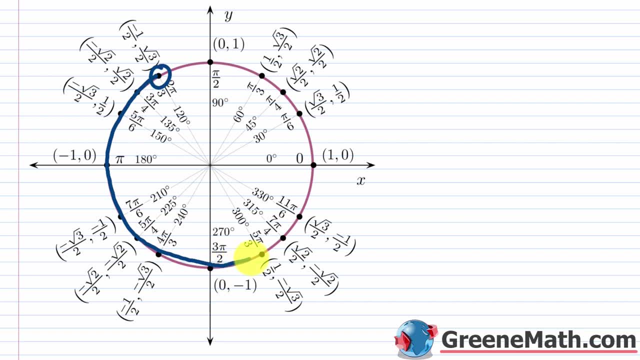 add pi, you're going to come into quadrant 4 and you're going to be at this 5 pi over 3.. So it should be true that the tangent of 2 pi over 3 is equal to the tangent of 5 pi over 3, because again, 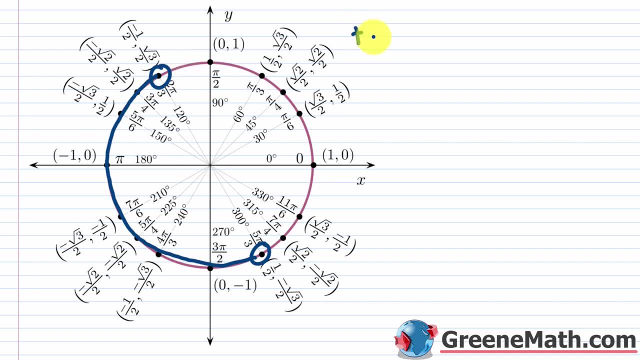 I'm coming back to the same tangent value. So let's just try that real quick. So we have the tangent of 2 pi over 3.. That would be equal to the sine of 2 pi over 3, which is the square root. 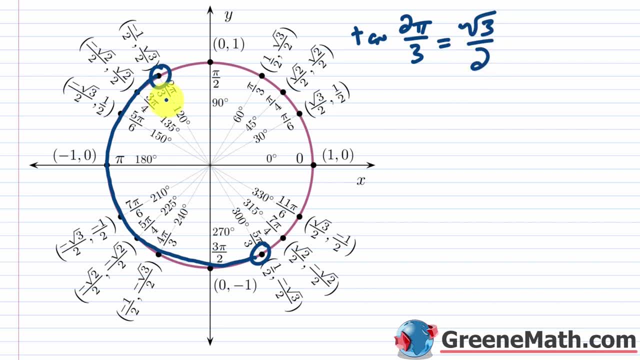 of 3 over 2.. And then divided by the cosine of 2 pi over 3, which is negative one half. So I'm going to multiply by the reciprocal, So times 2 over negative 1.. And of course the 2's are going. 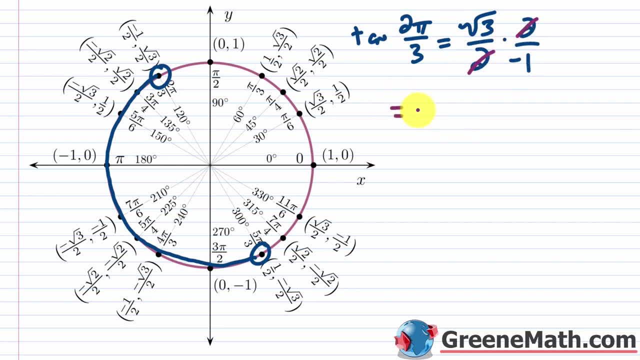 to cancel And you have square root of 3 over negative 1.. Let's just say that's the negative of the square root of 3.. Then if I come down here to 5 pi over 3. Again, if I look for the tangent of 5 pi over 3, it's going to be the same thing. I'm going to be. 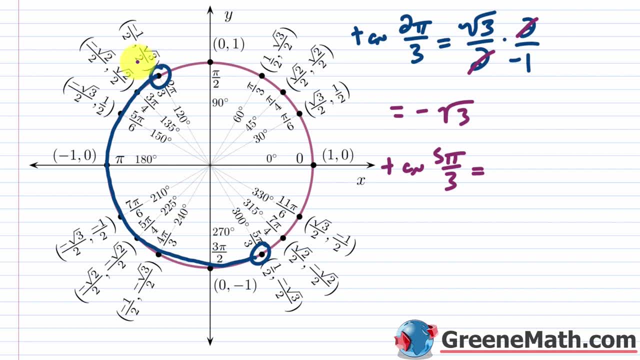 dividing opposites. Here it was basically a positive sine value divided by a negative cosine value, But here it's going to be a negative sine value divided by a positive cosine value. Well, we know if we have a positive divided by a negative or a negative divided by a positive. I'm going to 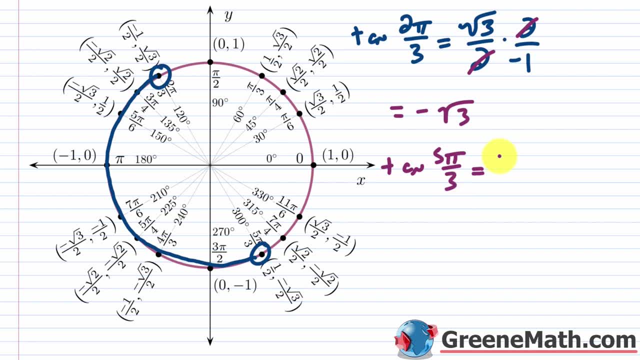 get a negative. So that's what's happening here. So this is just going to be my negative square root of 3 over 2.. That's the sine value here. So again, I'm going to multiply by the reciprocal, So times 2 over 1.. And let's go ahead and cancel. 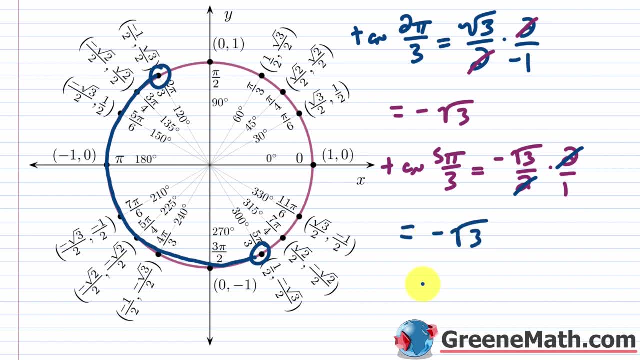 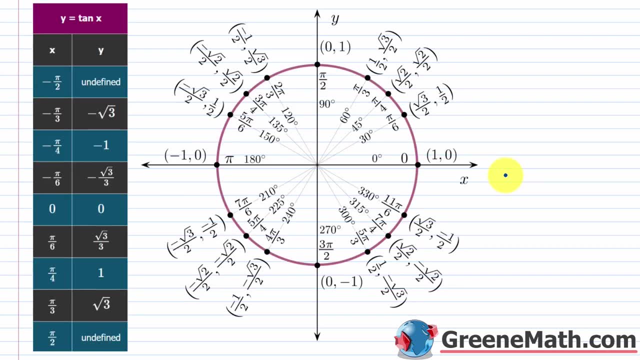 this with this, And so you get negative square root of 3.. So hopefully that gives you a little bit of insight into why the period is going to be pi. Alright. so what we're going to do now is just look at the basic graph for tangent. We're going to do this by grabbing some ordered pairs and just 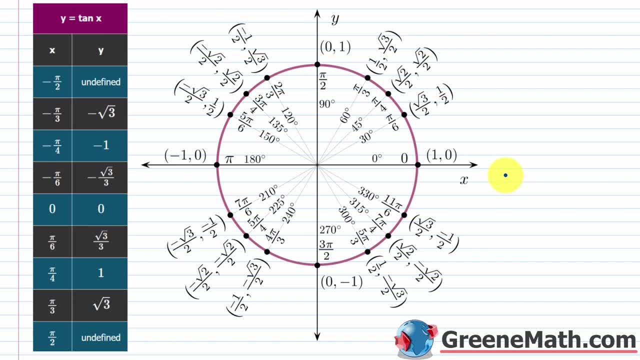 sketching this guy from negative pi over 2 to pi over 2, with both of those guys being excluded. I'm going to show you the graph. I want to cover a few things that basically cause a lot of confusion when you first see these graphs. The first thing is we should remember that when we see a negative 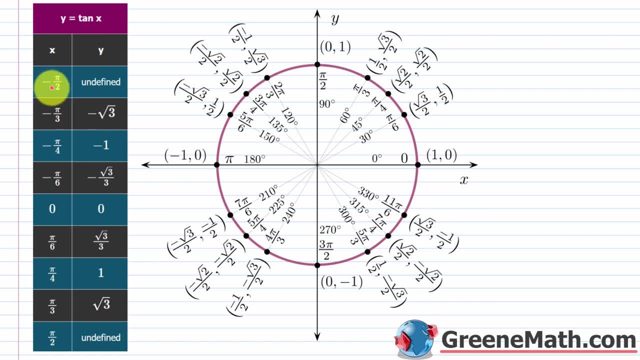 angle. we're rotating clockwise, In other words, something like negative pi over 2.. That means I'm starting here and I'm rotating clockwise. So it's going to be this guy right here. It would be coterminal with 3 pi over 2.. So this is negative pi over 2.. Now why does it say that it's undefined? 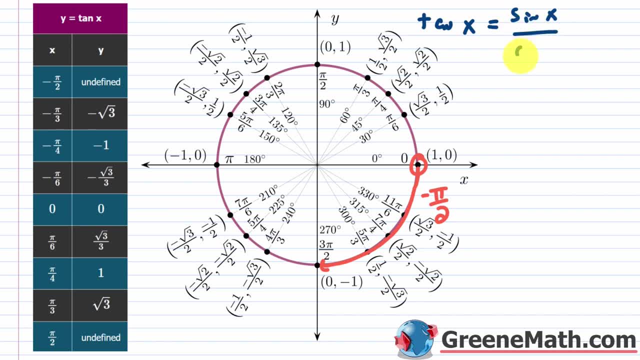 over 2?? Well, if I want the tangent of negative pi over 2, that would be equal to the sine of negative pi over 2 over the cosine of negative pi over 2.. Since this negative pi over 2 is coterminal with: 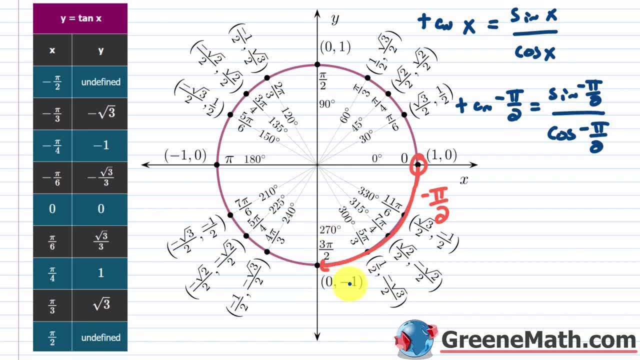 3 pi over 2. we could just take the value for sine and cosine from this guy right here, And so basically you could say that this is equal to the sine of negative pi over 2.. Well, that's negative 1.. Negative pi over 2.. Well, that's 0.. What do we know about division by 0? It's undefined, So basically, 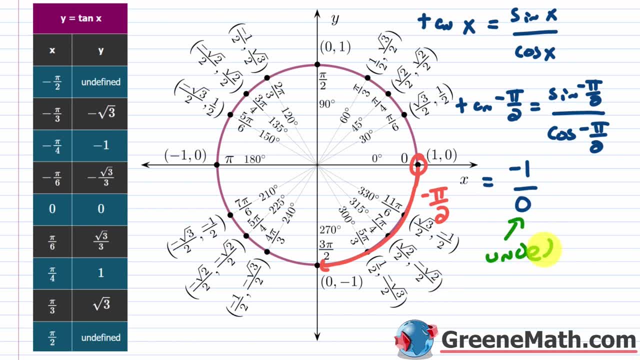 you stop at this point and you would say that this is undefined. Undefined, So this would always be true whenever the cosine value is 0. So basically, this is going to happen at pi over 2, then 3 pi over 2, then 5 pi over 2,, 7 pi over 2,, 9 pi over 2, so on and so forth. But also you have to consider: 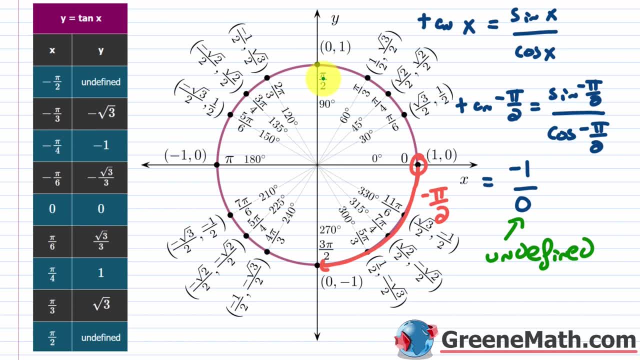 that would happen at negative pi over 2, negative 3 pi over 2, negative 5 pi over 2, so on and so forth. So a lot of books will cover this by saying that this guy is going to be undefined at odd multiples of pi over 2.. So that's a good way to remember it. You could also write it: 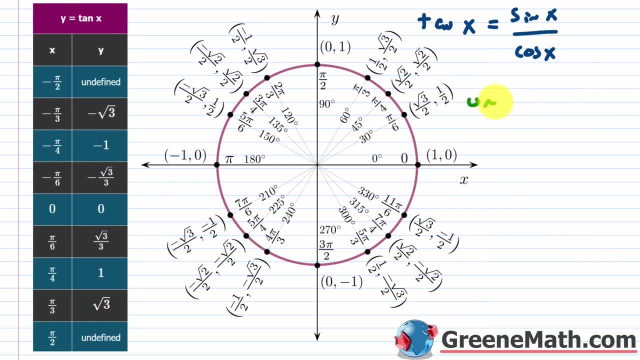 as, if you want to do it this way, you could say that it's undefined at pi over 2.. So this guy right here, plus pi n, where n is an integer. So basically, if it's a positive integer, then I'm rotating counterclockwise. So let's say: I add pi. 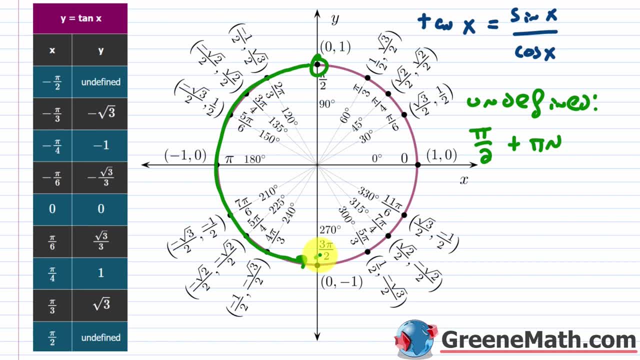 that's going to put me right here at 3 pi over 2.. And if I add pi again, then I'd be at 5 pi over 2, then 7 pi over 2, so on and so forth, If n was a negative integer. well then, basically now I have. 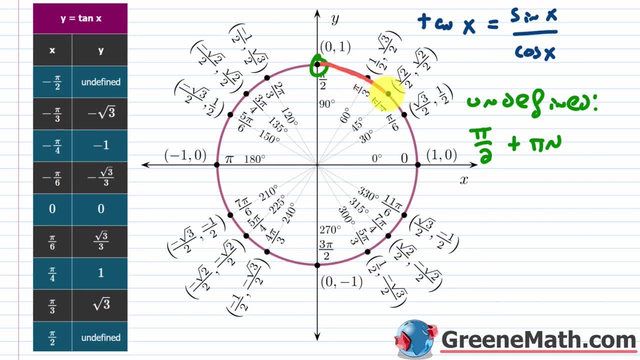 a clockwise rotation. So let's say I subtract pi and I rotate clockwise like this: Well now I'm not at 3 pi over 2, I'm going to be at negative pi over 2.. And if I do that again and subtract away another pi, well now I'm going to be at negative 3 pi over 2, and so on and so forth. 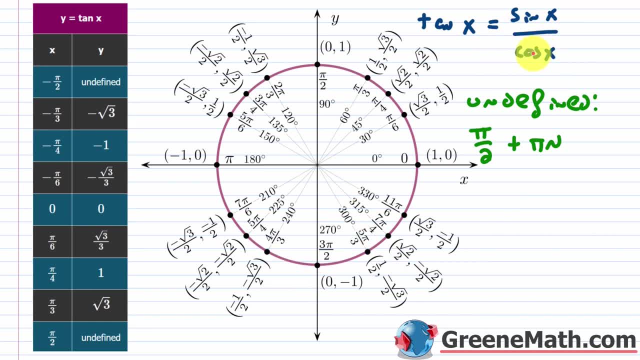 So all of those places it's going to be undefined because we're going to have a cosine value of 0 and division by 0 is undefined. Now the other thing you need to think about is that this guy is going to be 0 when the sine value is 0 and the cosine value is not 0. So something like, let's say: 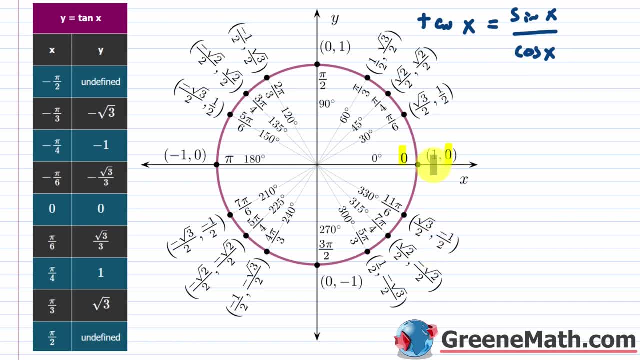 at 0 you have a sine value of 0 and the cosine value is 1.. Then at pi, you have a sine value of 0 and a cosine value of negative 1.. So basically for this you could say that the tangent value is going. 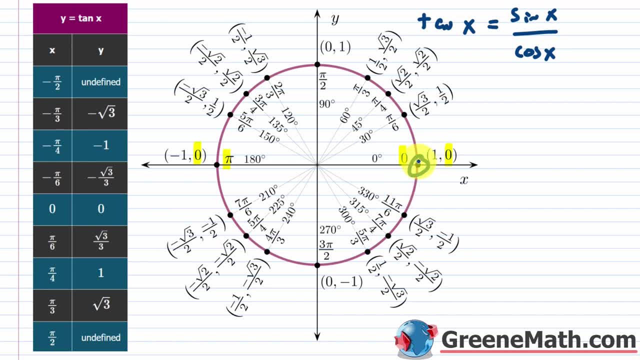 to be at pi n where n is any integer. In other words, you could start here and you could add pi and you would get to pi. You could add pi again and you would get to 2 pi and then 3 pi and then 4 pi, so on and so forth. And also if you wanted to start here and rotate clockwise. so if you 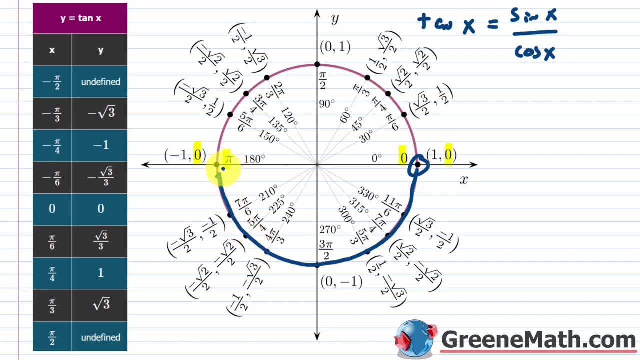 wanted to subtract pi away. well, now I'm going to be at negative pi, Then, if I do that again, I'm going to be at negative 2 pi, then negative 3 pi, so on and so forth. So basically, that's where. 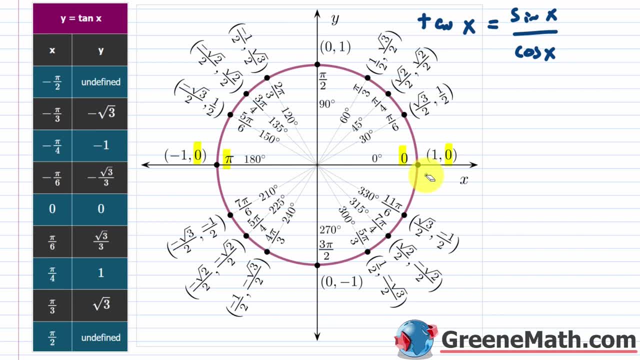 you're going to have a tangent value of 0, or you could say where you're at a tangent value of 0, intercepts going to be, And you can see on the table that we've made that we do have this 0 comma. 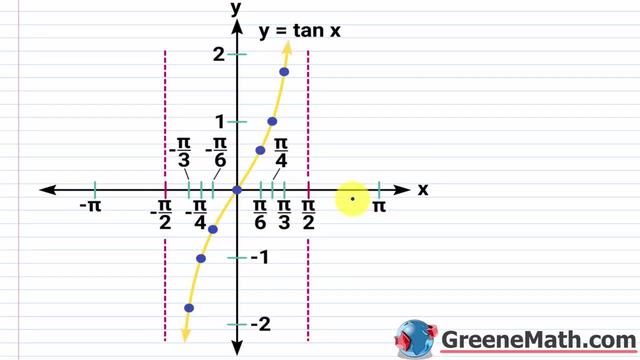 0.. Okay, so let's look at a basic sketch, for y equals tangent of x. So just using those points that we just had in our little table, So you have something like negative pi over 3 comma, negative square root of 3.. So that would be this point right here. Then you have negative pi over. 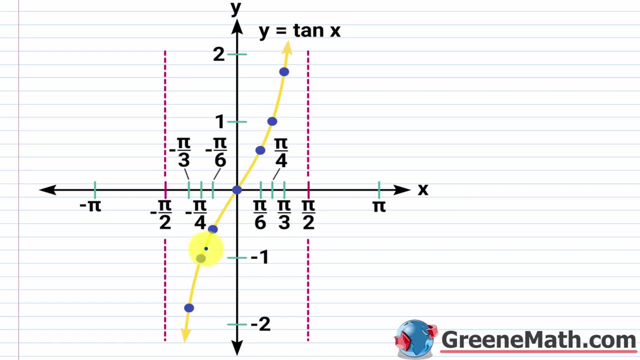 4 comma, negative 1.. So that'd be this point right here. So this point is actually one we're going to focus on. It'll be important for us later on. Then we have negative pi over 6 comma, negative 3.. So that's this point right here. Then we have our 0 comma 0.. So that's our x intercept And we'll 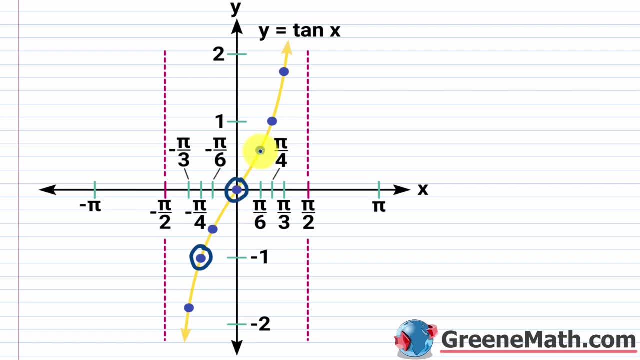 focus on that one later on. Then you have your pi over 6 comma, square root of 3 over 3.. Then you have your pi over 4 comma 1.. Again, this is one we're going to focus on, And then we have our 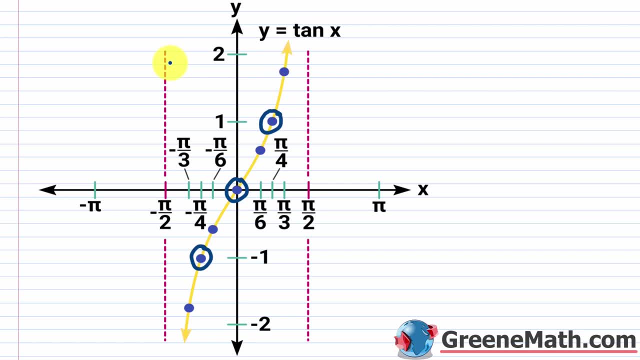 pi over 3 comma, square root of 3.. So that's going to be this guy right there. So one of the things to focus on here is you do have a vertical asymptote at this negative pi over 2 and then also pi over 2.. And that's being created because, again, at negative pi over 2 and pi over 2, you 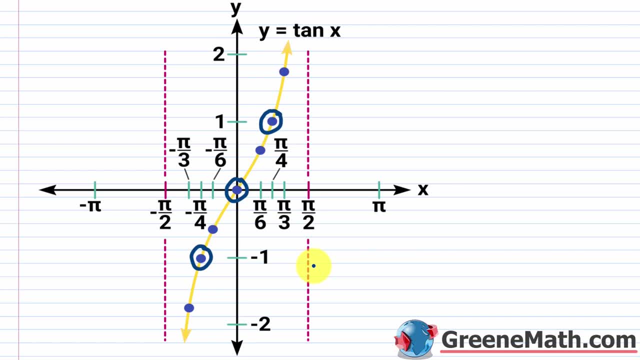 have division by 0, which is undefined. So we've seen this previously in our course. when we look at something like y equals 1 over x, We know that if you plugged in a 0 for x there, this is undefined. So if you look at the graph of that, you're going to end up with a vertical asymptote. 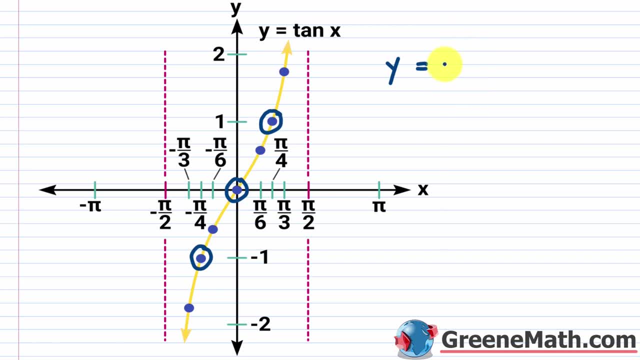 at x equals 0. So here, when you have y equals the tangent of x, the tangent of x, which you could really write as the sine of x, So the sine of x over the cosine of x. to make it more clear: Well, pi over 2 or pi over 2, something like that, 3, pi over 2,, 5, pi over 2,, 7, pi over 2, so on and so. 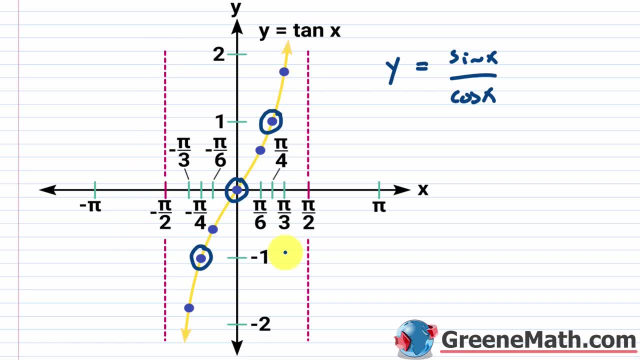 forth. Well, you're getting division by 0. So you're getting these vertical asymptotes. Now, when you think about the behavior, as this guy right here approaches pi over 2 coming from the left, So coming from the left, basically, as we approach this x value of pi over 2, this guy is 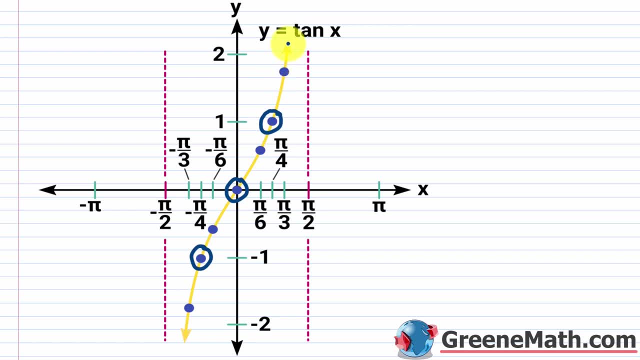 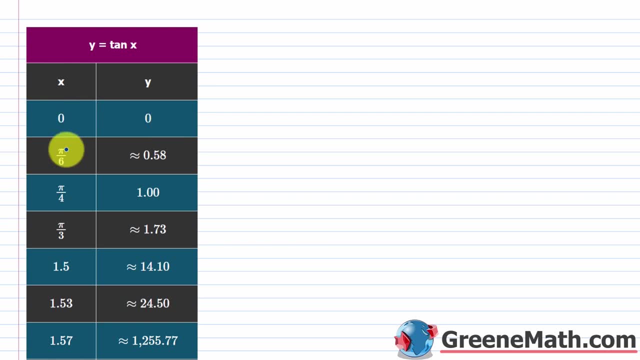 going to increase without bound, as they say. So approach positive infinity. So I have another little table for you. A lot of books will show this. So basically, at an x value of 0, you're going to get a y value of 0.. At pi over 6, you get about 0.58.. That's just approximating square. 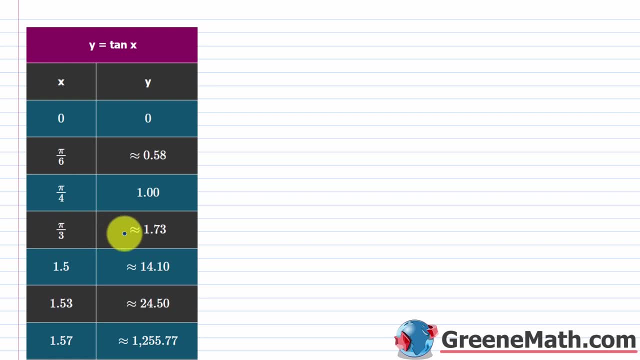 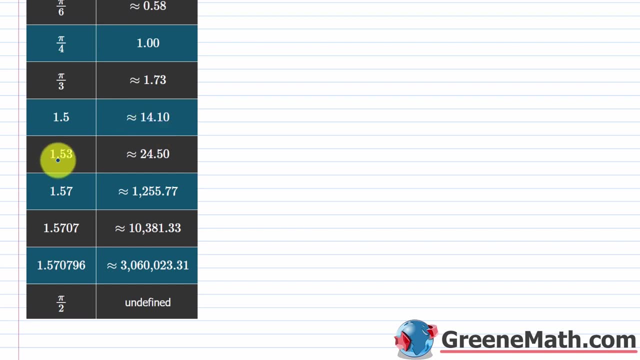 root of 3 over 3.. At pi over 4, you get 1.. At pi over 3, you get about 1.73.. That's approximating the square root of 3.. And then we have: 1.5 is about 14.10.. 1.53 is about 24.50.. 1.57 is about. 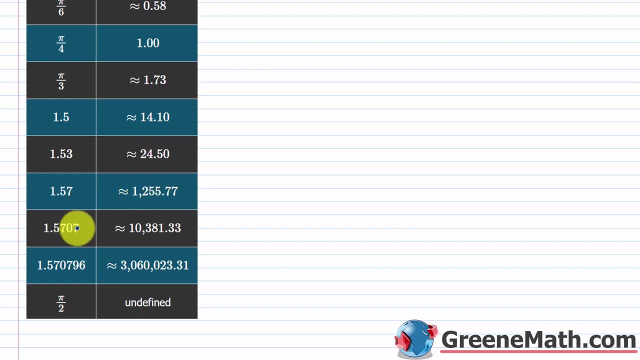 1,255.77.. And then this 1.5707 is about 10,381.33.. And then notice that as you get really close to pi- over 2. 1.570796,, you get 3,060,023.31.. So you can get as close to this as you want, You just can't. 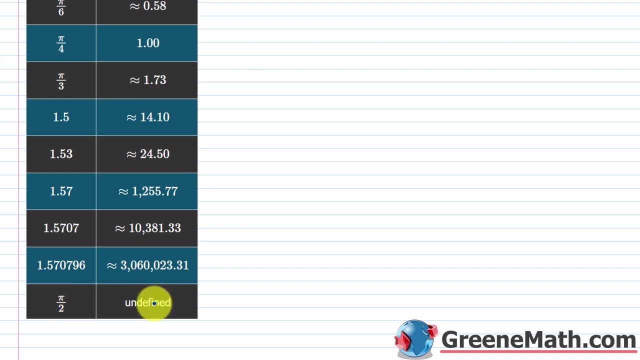 touch it, When you actually get to pi over 2, you're going to get undefined. But as you get closer and closer to it, this number is going to get larger and larger. So again, it's going to approach positive infinity, or what they'll say is increase without bound. Now, similarly as you, 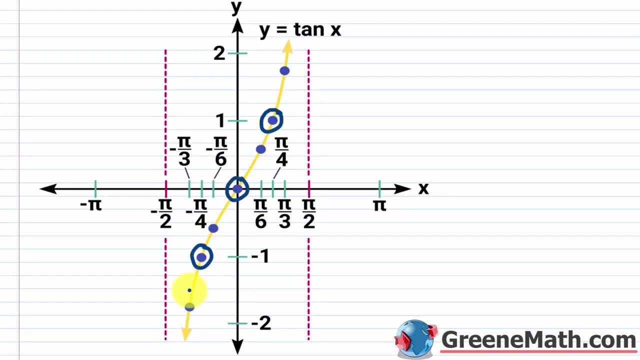 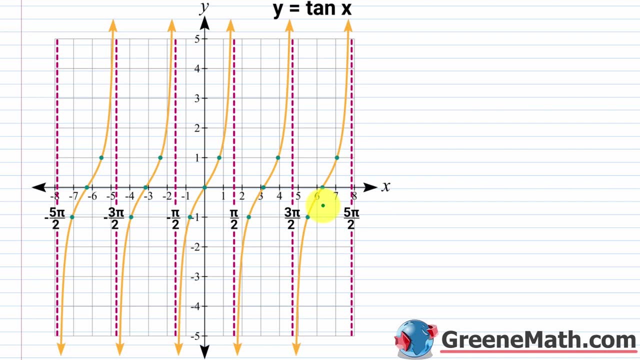 approach negative pi over 2 coming from the right. this guy is going to decrease without bound. So, basically, it's going to increase without bound And then, as you get closer and closer to it, this number is going to approach negative infinity. All right, So just like we saw with graphing sine or, 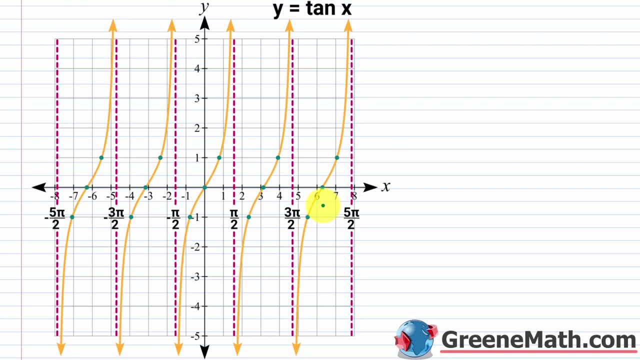 cosine. after we did one cycle of the graph, we were able to continue that to the left or to the right as much as we wanted. So here I have: y equals tangent of x. So I've extended this to the left and to the right a little bit, just so you can see a little bit more. So basically this is what we. 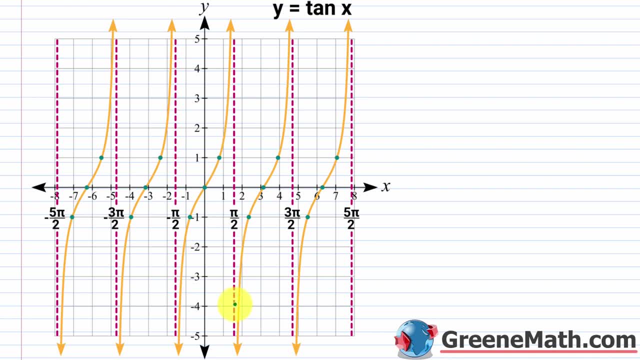 graphed already. So from negative pi over 2 to pi over 2, we see that we have a vertical asymptote at negative pi over 2 and then also another one at pi over 2.. So we're able to get a little bit more. 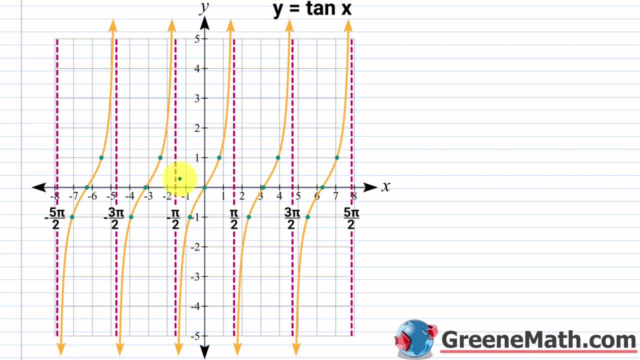 to. those are what we call consecutive vertical asymptotes. So when you graph a variation of y equals tangent of x- you're going to first find those guys- I'll tell you how to do that in a moment- And then basically you have these three points. So this one right here is at a quarter of. 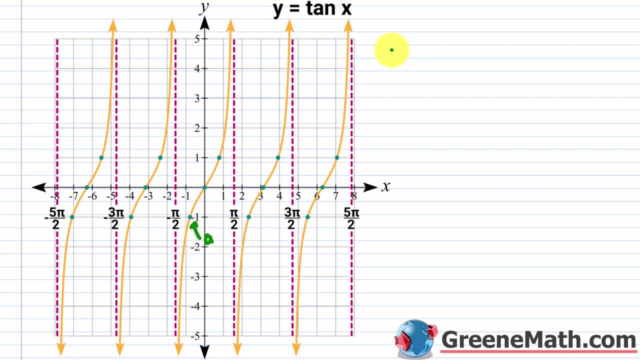 the way through, And let me just label this as a for right now. So a, let's just say that's negative pi over 4 comma, negative 1.. That's definitely something you want to memorize. Then let's call this b. This is going to be the halfway point, or the midway as a lot of people call it. So this is: 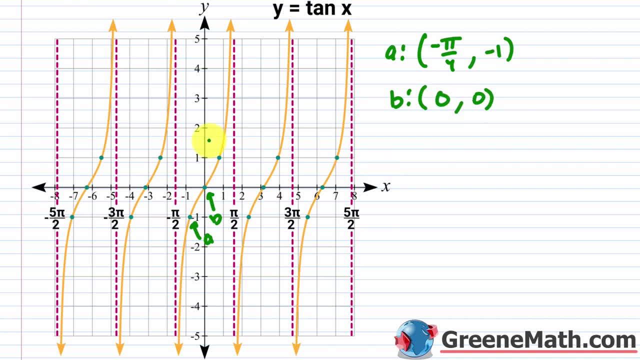 that's your x-intercept. So that's 0 comma 0.. And then let's call this point c, So that's three quarters of the way through. So basically that point is pi over 4 comma 1.. So you can use these: 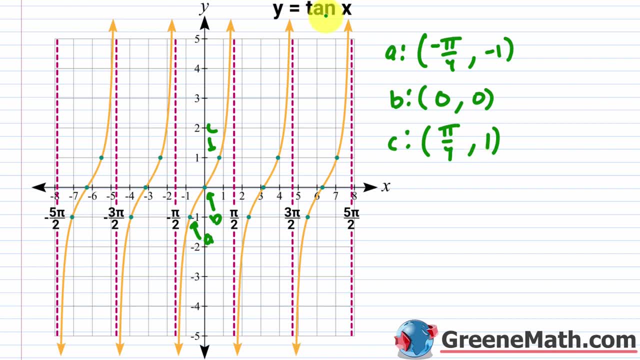 points. to basically graph: any variation of y equals tangent of x. If you want these points here or here or wherever it is, if you just want this one right here, remember the period for tangent is pi, So I could take the x value here. Let's just call this point d. Let's call this. 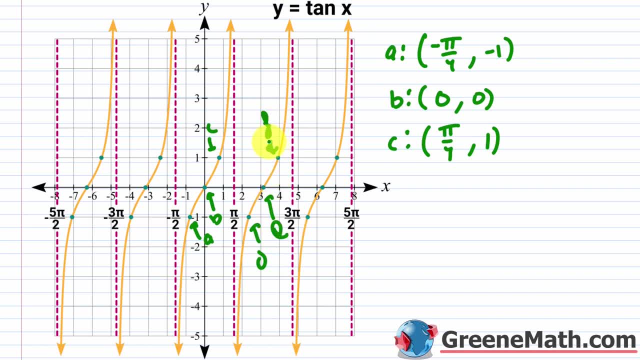 point e And let's call this point f. So if I wanted those, let's just go ahead and say that for point d. well, the y value is going to be the same. All I have to do is add pi to the x value, So negative. 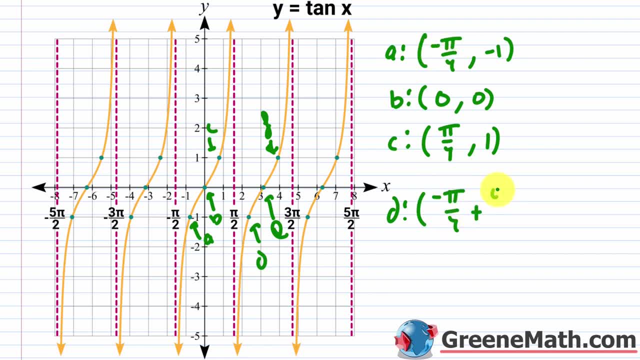 pi over 4, negative pi over 4 plus pi. So 4 pi over 4. to have a common denominator That's going to be 3 pi over 4.. So this would be 3 pi over 4 and then comma negative 1.. Then for e- I know that. 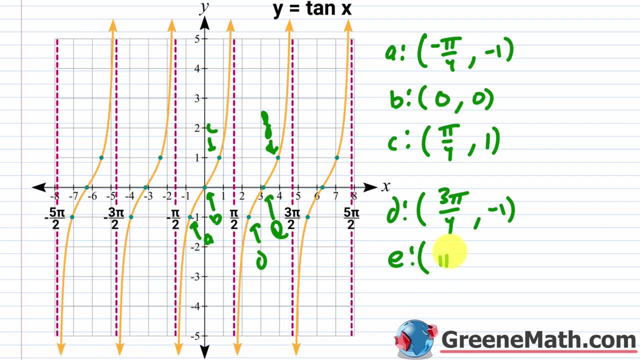 basically I would just take 0 and add pi, So that would be pi comma 0, y-coordinate things same, And then this is going to be for f Again. I'm just going to take this pi over 4.. So pi over. 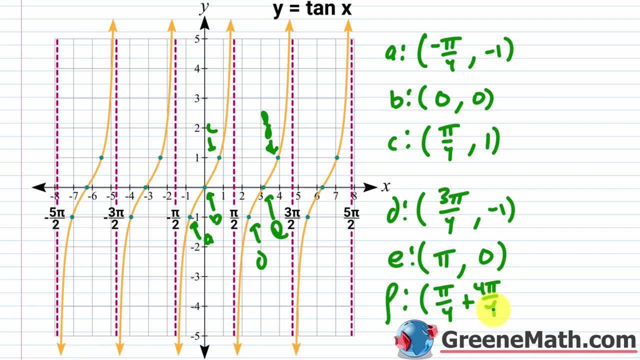 4.. I'm going to add pi, So 4 pi over 4.. So that's 5 pi over 4.. And then basically you're going to have the same y-coordinate, So it's still going to be 1. And you can basically use that process. 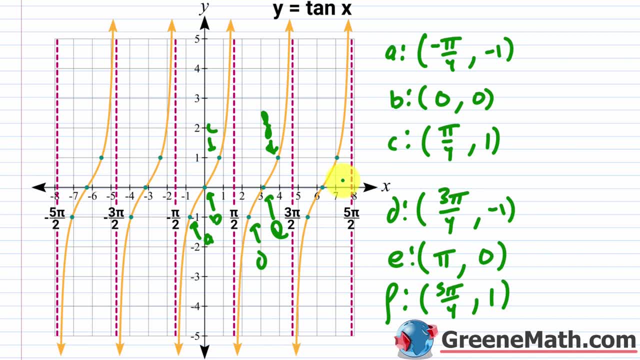 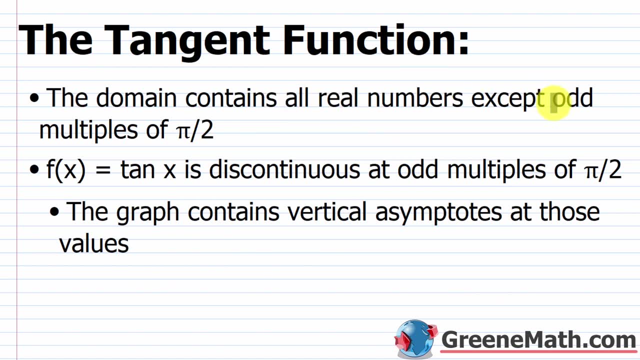 to extend the graph to the left or to the right as much as you want, All right, so just some information that you need to know. So for the tangent function, the domain contains all real numbers except odd multiples of pi over 2.. Some books will write that as pi over 2 plus pi n, where n is an integer. 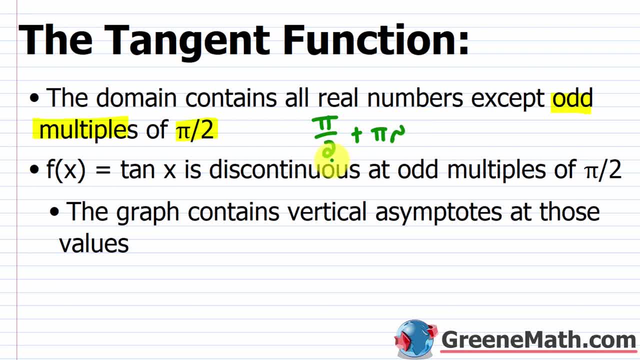 So basically it's just telling you things like pi over 2,, 3 pi over 2,, 5 pi over 2,, 7 pi over 2.. You could also have negative pi over 2, negative 3 pi over 2, so on and so forth. We have f of x is. 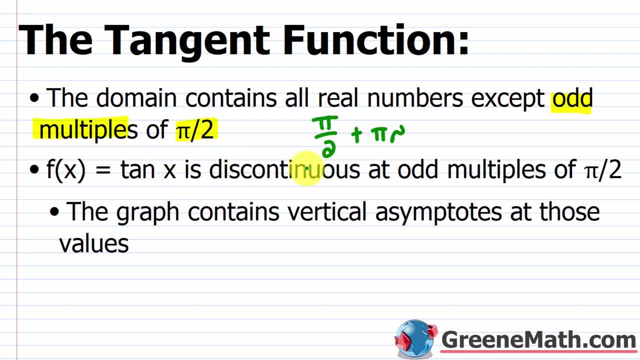 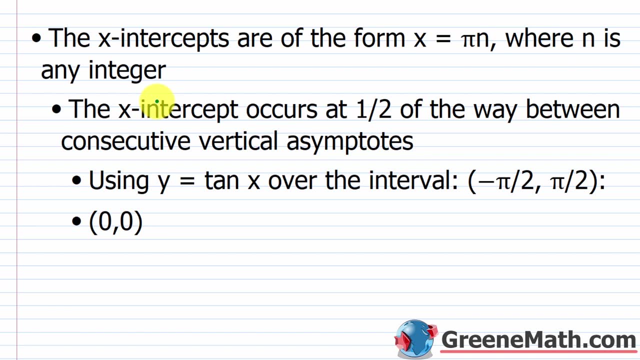 equal to tangent of x. You can also write: y equals tangent of x is discontinuous at odd multiples of pi over 2.. So basically, we've seen that the graph contains vertical asymptotes. at those values, The x-intercepts are of the form: x equals pi, n where n is an integer. We know that. that's because that's where the sine 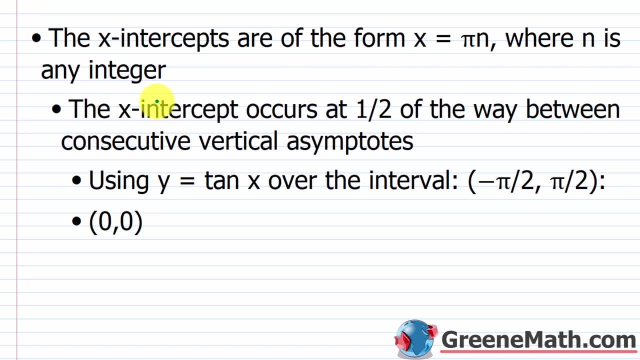 values are 0. And 0 divided by something that's not 0 gives you 0. So that's why that occurs. The x-intercept occurs at half of the way between consecutive vertical asymptotes. So if we're using y equals tangent of x over that interval that we talked about. so from negative pi over 2 to pi. 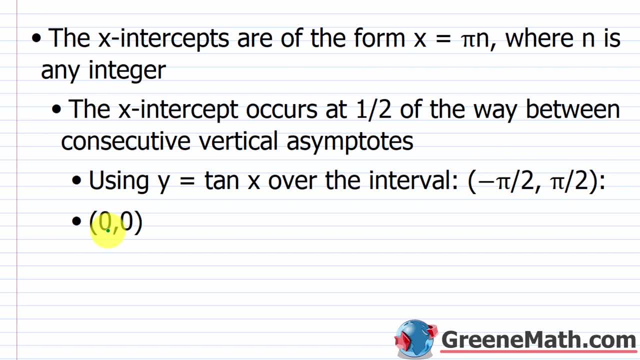 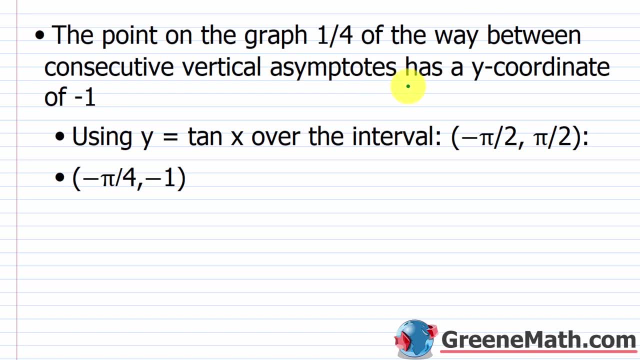 over 2, with both being excluded, that's going to occur at 0 comma 0.. Then we have our point on the graph. that's a fourth of the way between consecutive vertical asymptotes. This is going to have a y coordinate of negative 1.. So, again using that example, y equals tangent of x. 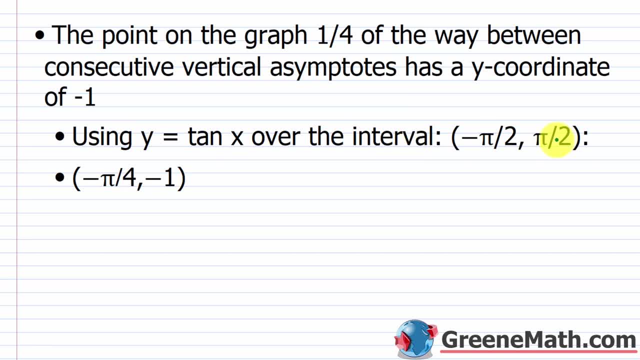 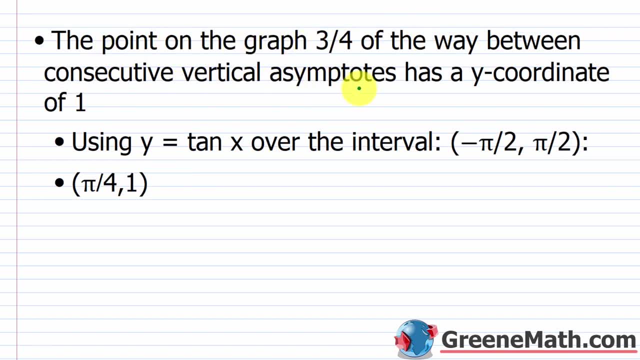 over the interval from negative pi over 2 to pi over 2, both excluded, we have that negative pi over 4 comma, negative 1.. And then the point of the graph three-fourths of the way between consecutive vertical asymptotes has a y coordinate of 1. So again, using y equals tangent of x over that. 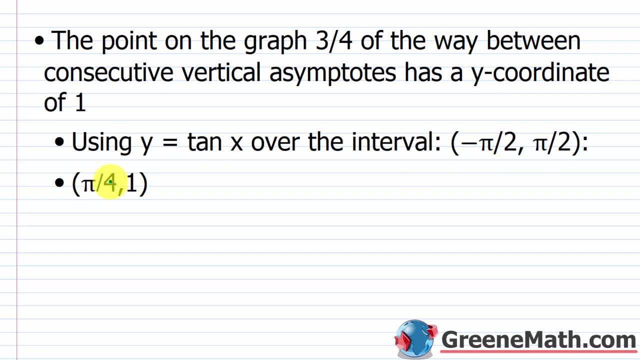 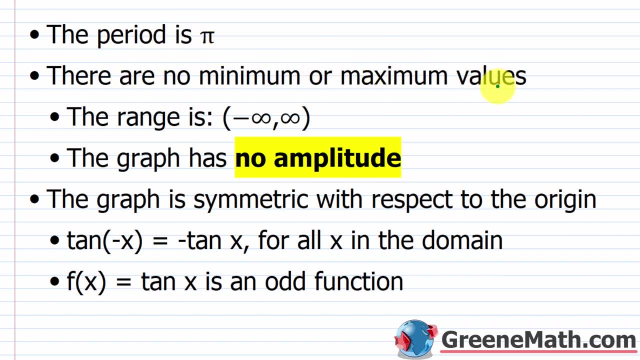 interval: negative pi over 2 to pi over 2,, both being excluded. we have that pi over 4 comma 1.. So we already know that the period is pi, And then there are no minimum or maximum values. So that's important. We saw that the range is from negative infinity to. 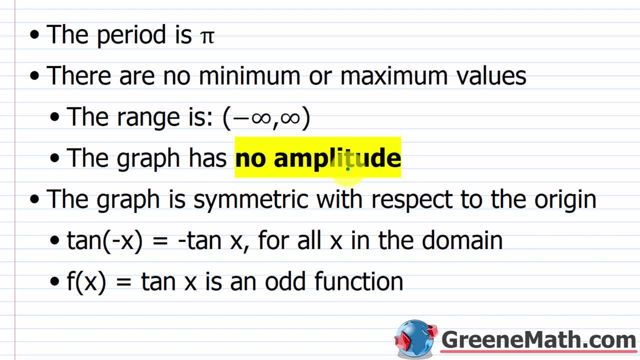 positive infinity. So that tells us that the graph has no amplitude. So that's important because you might get that on your test. It might ask you for the amplitude. Remember that when you think about the amplitude we learned in the last lesson- when we're graphing sine and cosine, that's half the 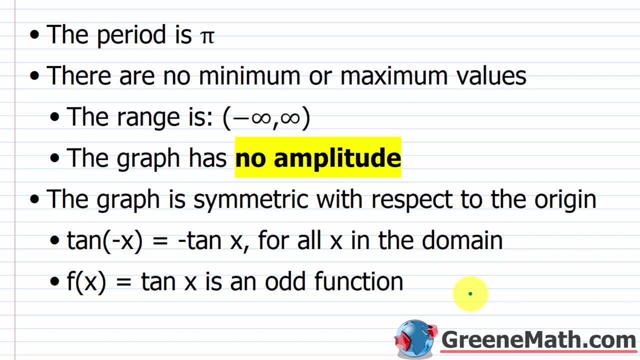 difference between the maximum and minimum values. Well, here again, there are no minimum or maximum values, So you're not going to have an amplitude here. Then we can also say: the graph is symmetric with respect to the origin. Remember that tells us we have an odd function, So the 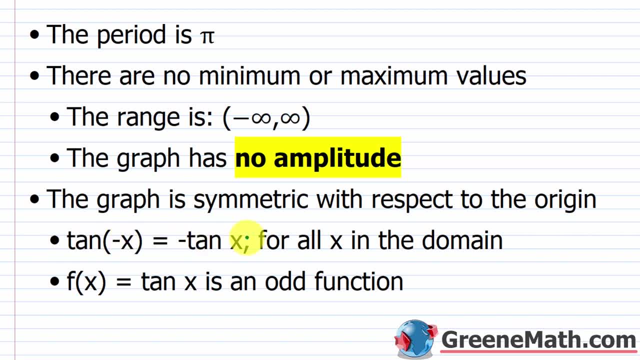 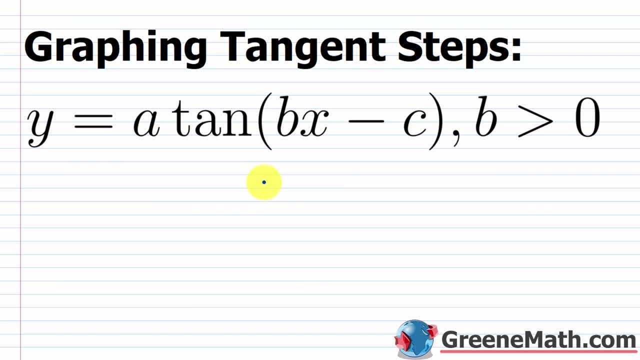 tangent of negative x is equal to the negative of the tangent of x. for all x in the domain. Again, f of x equals the tangent of x is an odd function. All right, let's talk about the steps involved with graphing the tangent function. So what I'm going to do is give you a simple model here, And 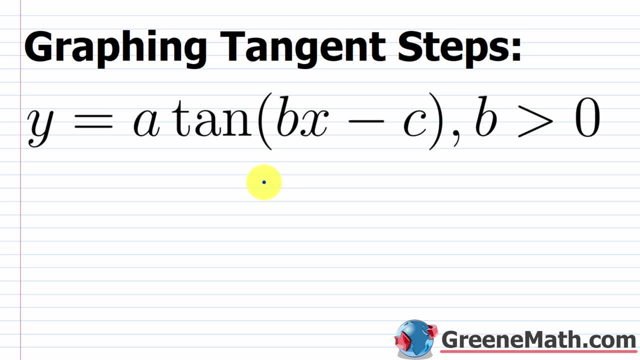 then if we get something that's a little bit more challenging, we can just modify our steps. So the first thing is we have y equals a times the tangent of bx minus c, And we're specifically going to say here that b, which is the coefficient of x, is greater than. 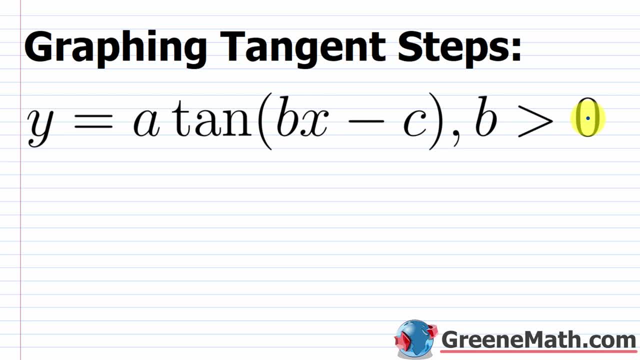 zero. Of course, we'll see scenarios where b is negative, And I'll show you how to deal with that with identities. For right now, let's go ahead and talk about the period. So what is the period? Again, when we think about this, from our sine and cosine lesson, we know that if we had something, 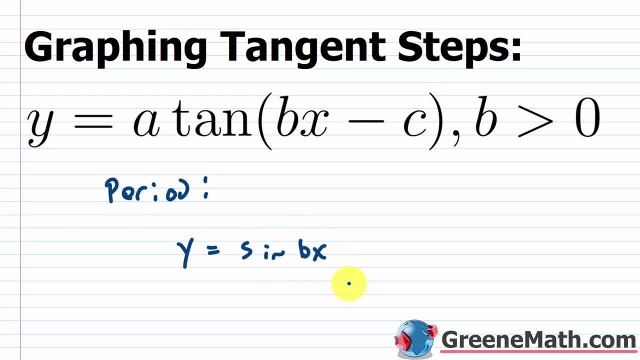 like y equals the sine of bx. well, the period here, so the period here, was the standard period, which is 2pi divided by b. Well, it's a similar thought process here. When you have y equals the tangent of x, the standard period is now pi, Not 2pi but pi. So let me put that off to the side. 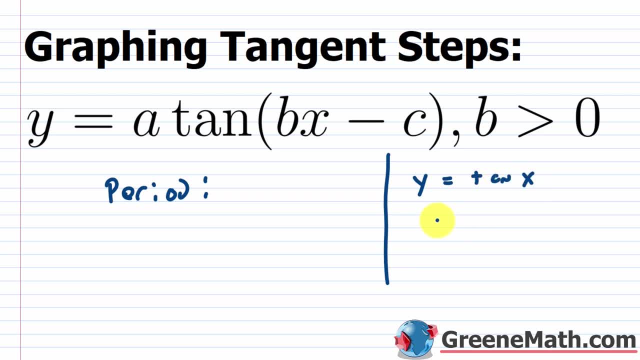 So y equals the tangent of x, the period is pi. So we know that. Well, here the period for this guy right here. because you have b that's multiplying x, it's going to be pi over b. Now I have a little. 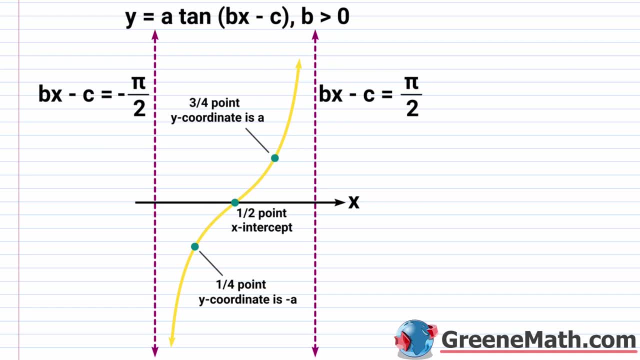 sample illustration here to go through. We'll take a look at that, but first we have to make some go through the procedure. So basically, the first thing you're going to do, you're going to find these two consecutive vertical asymptotes, And the way you do that is you go back to again. 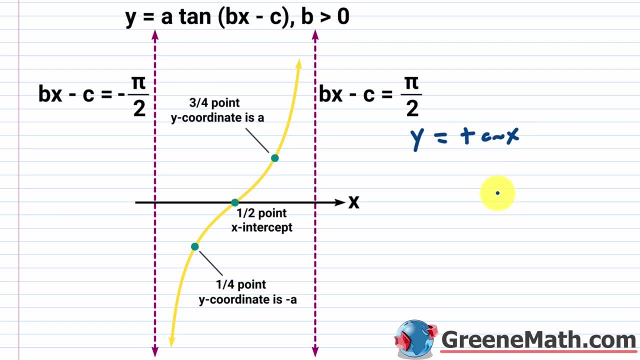 y equals the tangent of x. We know that we generally graph one cycle from negative pi over 2 to pi over 2, with both being excluded. So you have x equals negative pi over 2 and you have x equals pi over 2.. So you could say that one cycle occurs where x is greater than negative pi over 2. 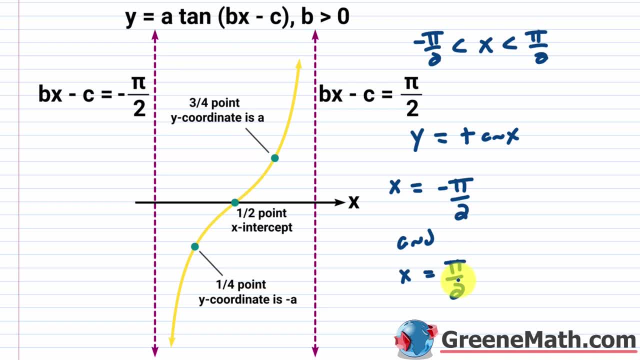 and less than pi over 2.. So this negative pi over 2 and pi over 2, those are consecutive vertical asymptotes. Now we don't have an argument of x, we have an argument of bx minus c. So we just have to adjust this. Let me get rid of this real quick. We're going to use the same thought. 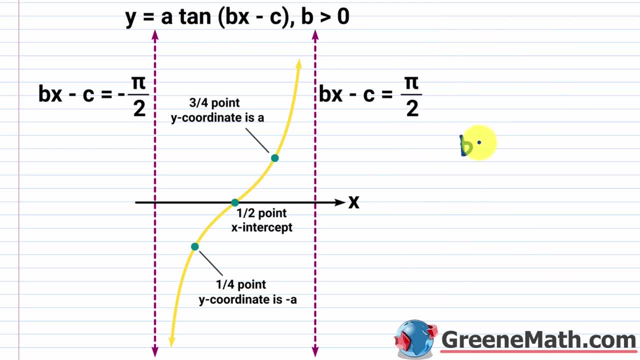 process, though We're going to say that we're going to do one cycle where bx minus c is greater than negative pi over 2 and less than pi over 2.. And we can find the vertical asymptotes by saying that bx minus c is equal to negative pi over 2 and less than pi over 2.. And we can find the 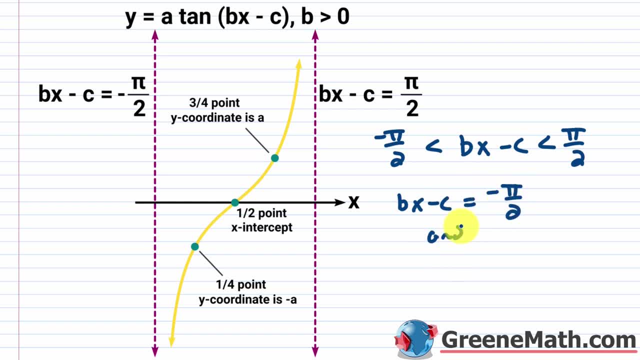 vertical asymptotes by saying that bx minus c is equal to negative pi over 2.. So that would be one of them And we'll put: and bx minus c is equal to pi over 2.. So that would give you this guy and this guy, So the two consecutive vertical asymptotes that you're looking for Once you. 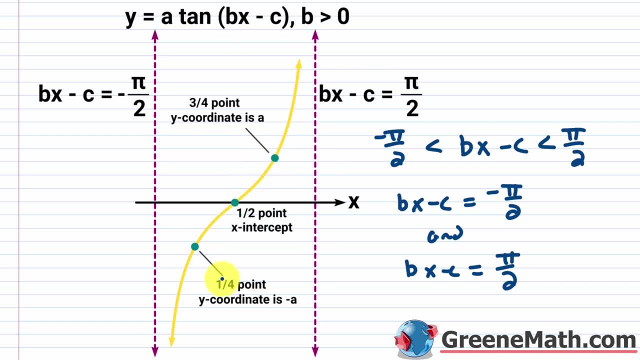 have that. you need to find these three points. So you're going to have one that's a quarter of the way, halfway and three quarters of the way. The way you do that is you find your quarter period, just like we did with sine and cosine, And so, basically, if the period is pi over b, 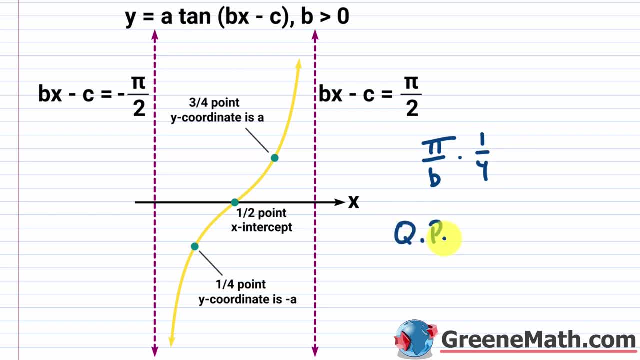 well, you can multiply that by a fourth And you could say that the quarter period is going to be pi over 4b. So you take your leftmost vertical asymptote, So that's x equals some number. you take that value and you add pi over 4b to that And you're going to get the x value for the. 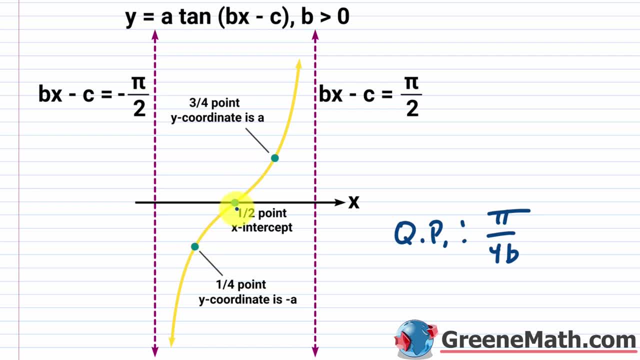 quarter of the waypoint, then you add the quarter period, you get the halfway point, then you add the quarter period, you get the three quarters of waypoint And you could add a quarter period to get the next vertical asymptote if you wanted to. But again, you should already know what. 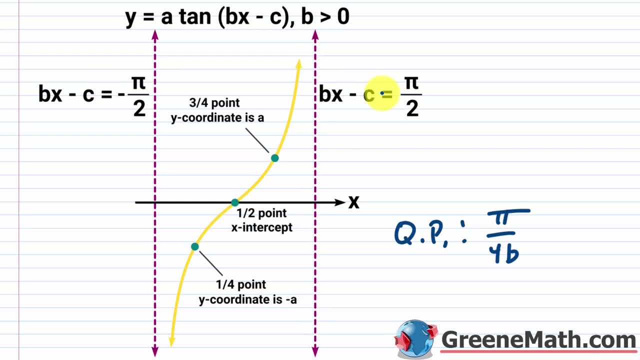 that is because you already set up those two equations. So the main thing is that you just have to find the x values there. the y values are very easy to find. you can just use the fact that at a quarter of the way through the y coordinate is negative a. So whatever this is, it's the 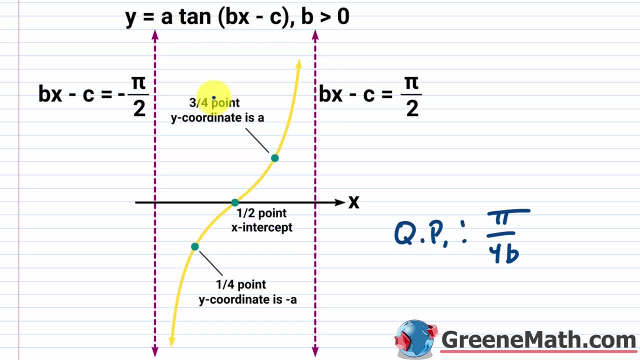 negative of it: halfway through it's going to be zero, and then three quarters of the way through is just going to be a. Again, going back to what we saw earlier when we did: y equals the tangent of x. remember I told you to memorize these three points. you have negative pi. 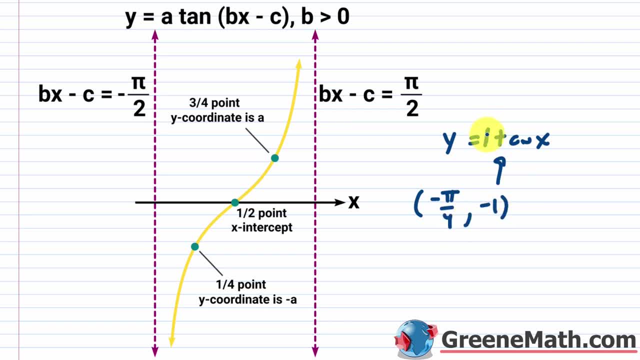 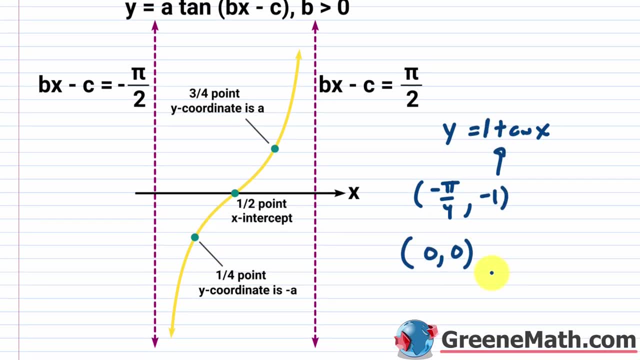 over four comma negative one. Well, you could put a one here, if you want, for clarity. what's the negative of one? that's how you get that y coordinate. then you have another point which is zero comma zero. that's just your x intercept. And then you have another point. 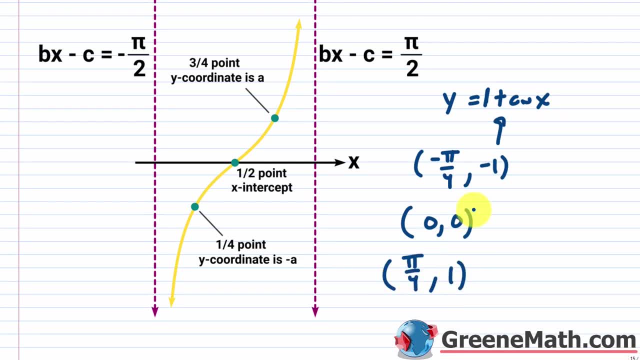 which is pi over four comma positive one, Okay, so positive one there. So I would just memorize those three points from this basic tangent function. If you do that, you're going to be good to go with any graph that you come across. All right, let's take a look at an example. 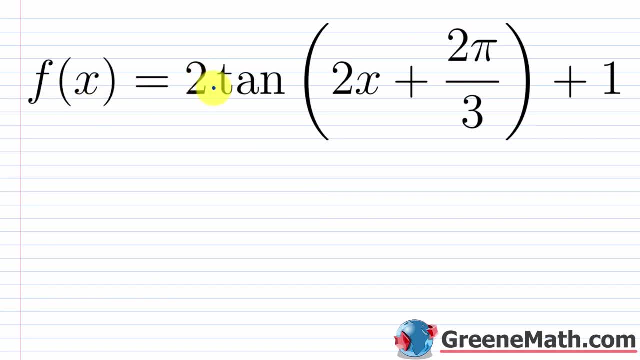 with the tangent function. So we have f of x equals two, and then tangent of two x plus two, pi over three and then plus one. So what I'm going to do is just use the procedure that we just talked about. There's alternative approaches When I get done with 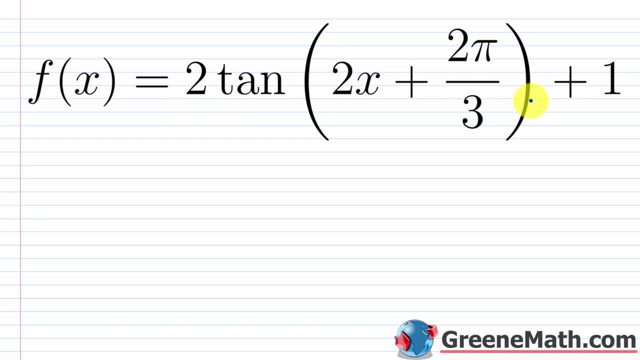 this problem. I'll show you another way that you could do it. I'll just do a few points using graphing transformations only. The first thing is to think back to what we talked about a moment ago. If we're graphing something like, y equals the tangent of x, generally speaking. 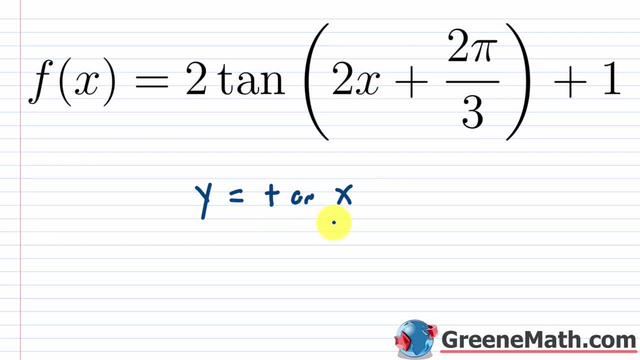 if you're graphing that over one period, or if you say you want to graph one cycle of this guy, well, we know that we're going to do. x is greater than negative pi over two and less than pi over two. We know there's a vertical asymptote at negative pi over two. 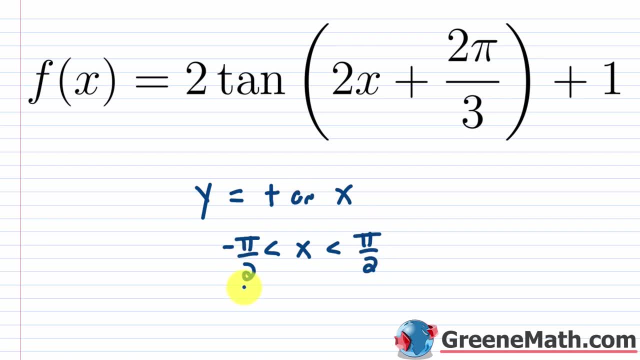 and also at pi over two, because again the tangent of negative pi over two and the tangent of pi over two is going to be undefined, because we'd have division by zero. So what you want to do is set up an inequality. here The argument is not x like we have here, The argument is two x. 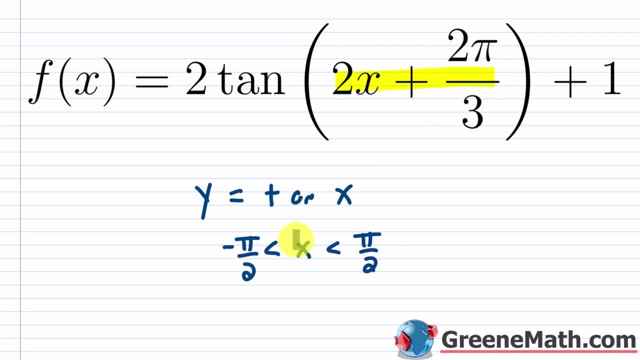 plus two pi over three. So this guy right here just gets plugged in for this right here. So you're going to set up the inequality. let me get rid of this where you say two x plus two pi over three is greater than negative pi over two and less than pi over two, And I'm just leaving myself. 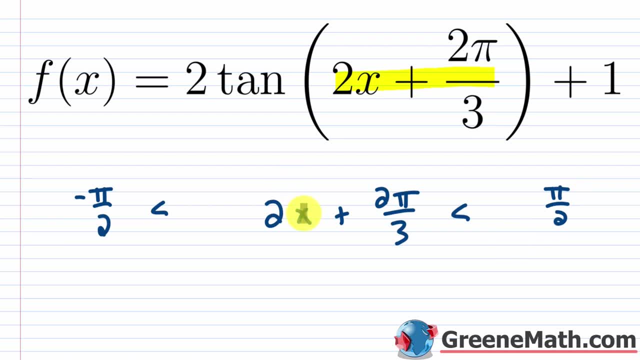 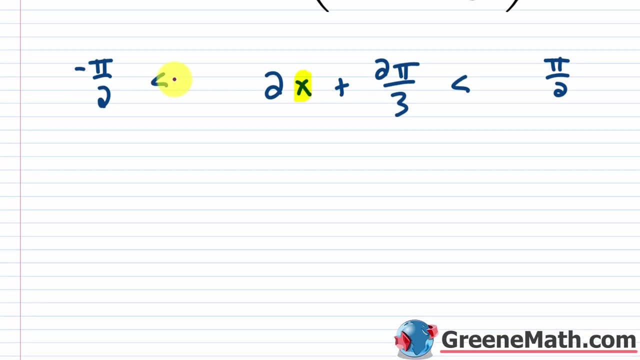 some space because we're going to multiply them up. So we're going to solve this inequality for x. So this is the goal right there. So we do have some fractions involved. I would personally like to clear those. Some people don't mind them, but I find that working with fractions is very tedious. 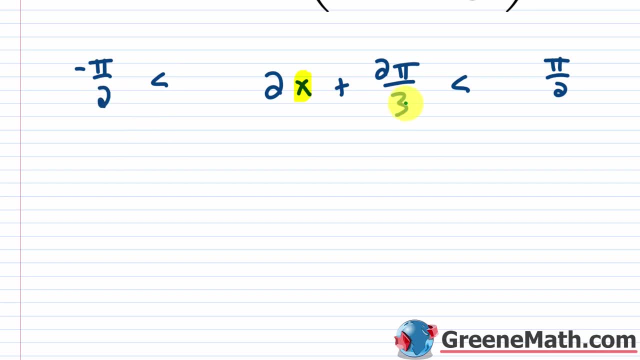 So what I would do is look at the denominator here of 2, then you have a denominator of 3, then a denominator of 2.. So the least common denominator is going to be 3 times 2 or 6.. So just multiply each part here by 6, and then you can get. 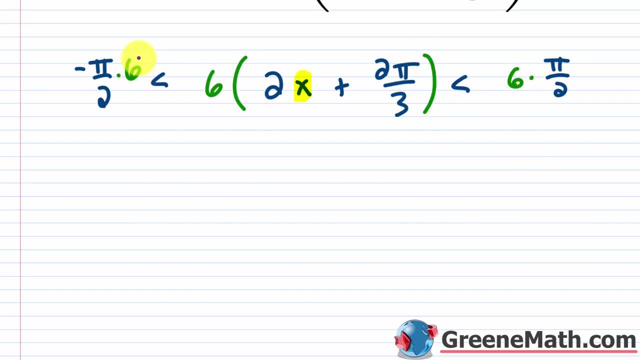 rid of the fractions and you won't have to deal with them. So basically, 6 divided by 2 would be 3. And so you'd have negative 3 pi there. So this is less than This gets distributed to each guy. 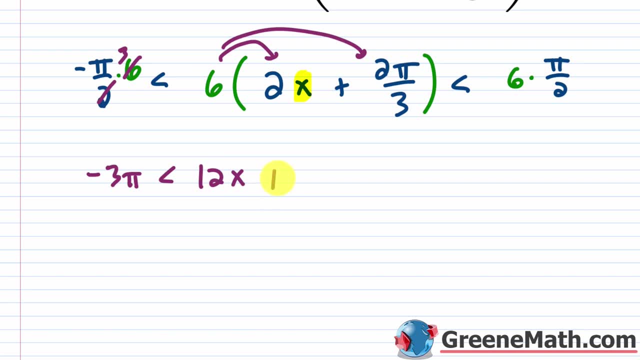 So 6 times 2x is 12x, And then plus you have 6 times 2 pi over 3.. So this 6 would cancel with this 3 and give you a 2.. 2 times 2 pi is 4 pi. So let me write that there And then basically: 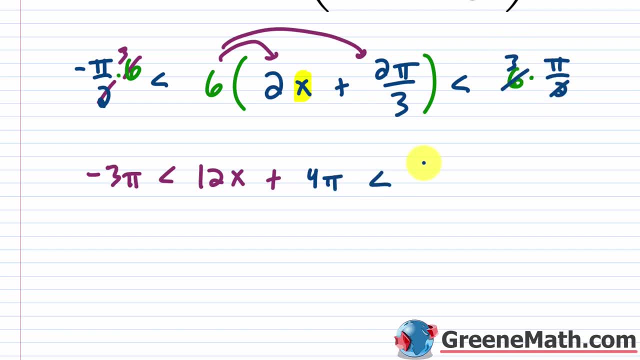 this is less than 6, would cancel with the 2 and give me a 3.. So 3 times pi is 3 pi. At this point again, if you're trying to isolate x, what I would do is subtract 4 pi away from each part. 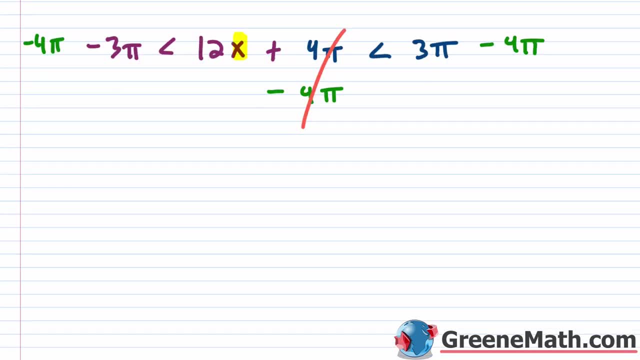 So let me do that over here. So let me do that over here. On the left, you have a negative 4 pi minus 3 pi, That's negative 7 pi. This is less than In the middle. you're going to have 12x, which is less than On the right. you're going to have 3 pi. 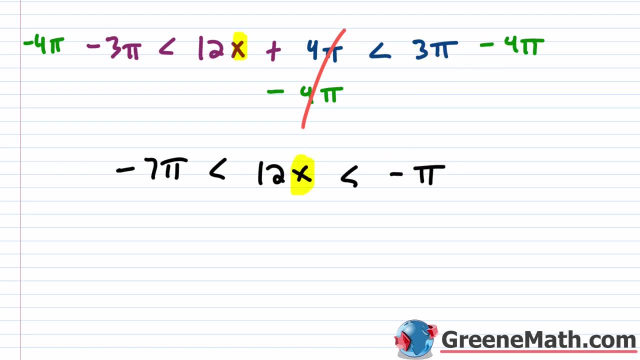 minus 4 pi, That's negative pi. Again, if you want to isolate x in the middle, just divide each part by 12.. So divide by 12,, divide by 12, and divide by 12.. So this right here is going to cancel. 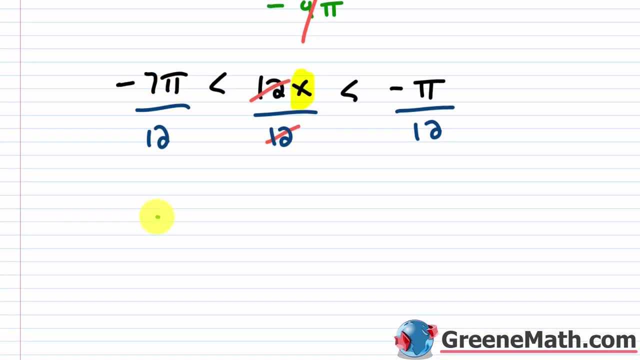 Let me slide down here a little bit. And you're going to have negative 7 pi over 12 on the left, And this is less than x, which is less- Then negative pi over 12.. So this is telling me that my function is going to go through one cycle from negative 7 pi over 12. 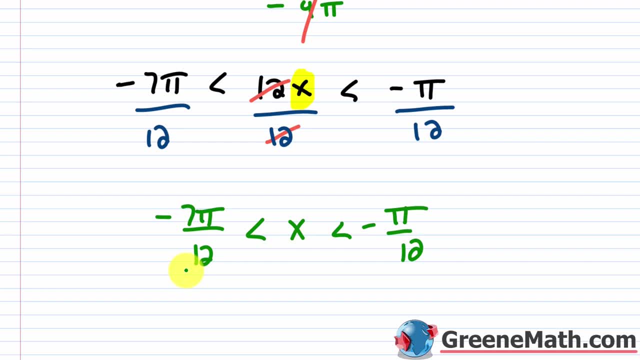 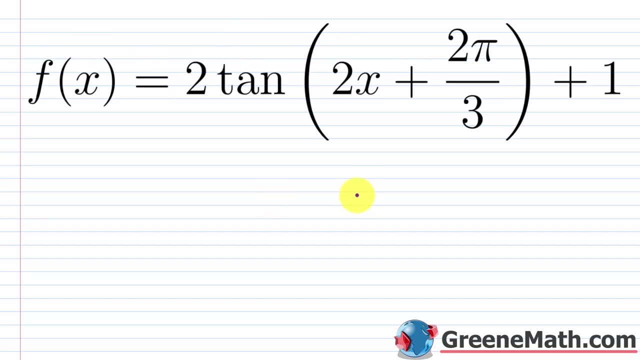 to negative pi over 12, where negative 7 pi over 12 and negative pi over 12 are my two consecutive vertical asymptotes. And let me come down to this page right here. Let me go back up and let's talk about the period. So what is my period? And then I'm also going to need to know what is my quarter. 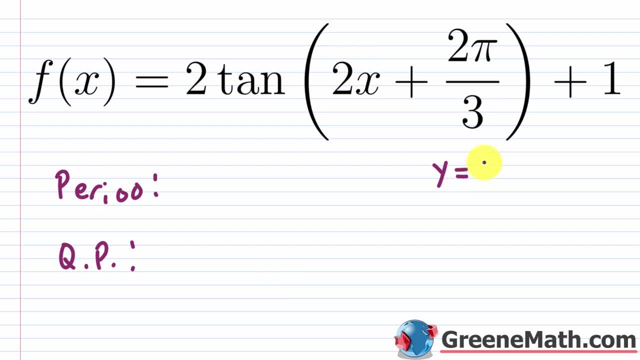 period. So the period again, if you're looking at, y equals the tangent of x. well, the period is just going to be pi. If I change this to y equals the tangent of bx. well, now, provided that b is positive. again, if you don't have a positive b, 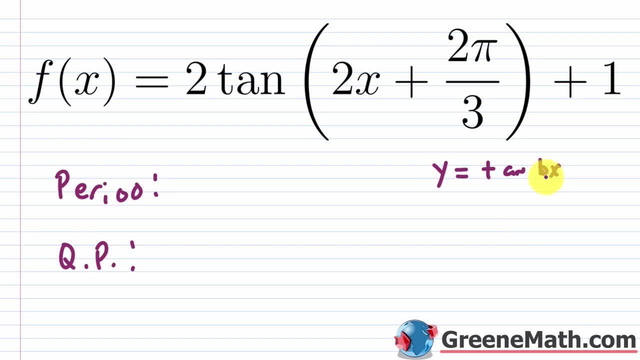 you could just use absolute value bars. But provided that b is positive, you'd say the period is pi over b. So you're just dividing by whatever the coefficient of x is. So here we have a coefficient of x that's 2.. So the period is pi over 2.. And then the quarter period. 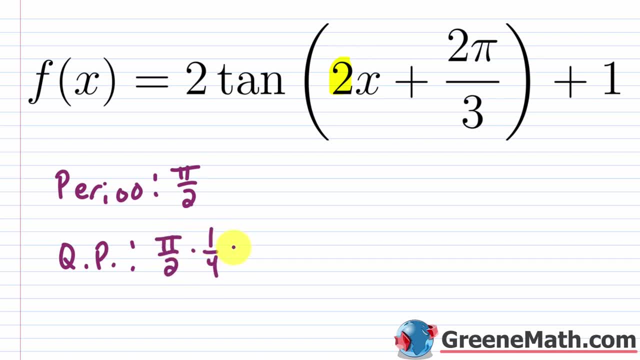 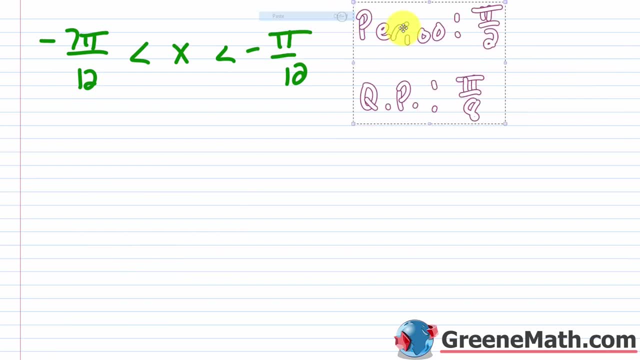 is pi over 2 times a fourth, So that's going to be pi over 8.. So this is pi over 8.. If you want to know if you've got the right period, let's come down here and paste this in and just put a little border around it. you can actually subtract, So you're. 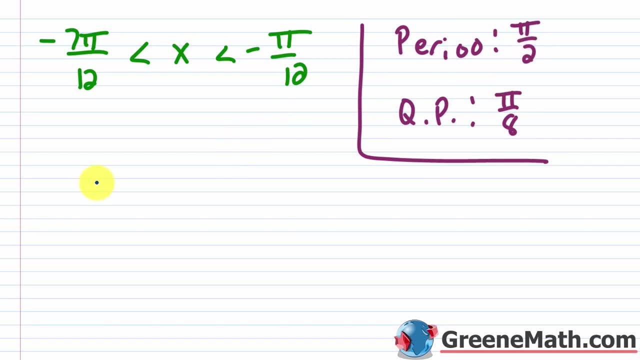 going to go larger minus smaller and you should get pi over 2. So negative pi over 12.. So that's for this guy right here. And then you're going to go minus this negative 7 pi over 12.. Convert this. 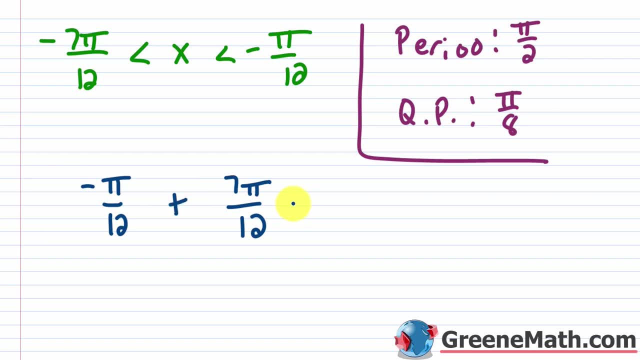 into plus Minus a negative is plus a positive. So this becomes you could write negative 1, there, So negative 1 pi plus 7 pi, that's going to be positive 6 pi over 12.. And of course, 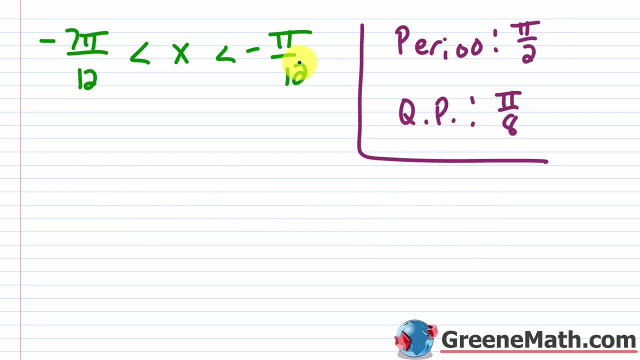 this simplifies to pi over 2.. So that confirms the period, right there. So you have two consecutive vertical asymptotes. We put vertical asymptotes here You have one at x equals negative 7 pi over 12.. And then the other I'll just put, and here x is equal to negative pi over 12.. 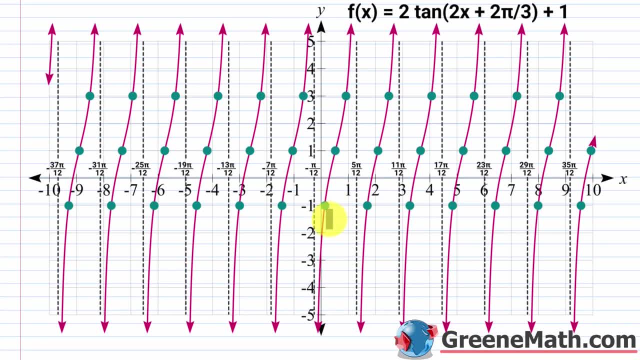 If you come to the graph- and I have a link for you on Desmos. if you want to get something that has more detail, I have all the points labeled for you If you want to click on that. This is what we've found so far. So this is the vertical asymptote. 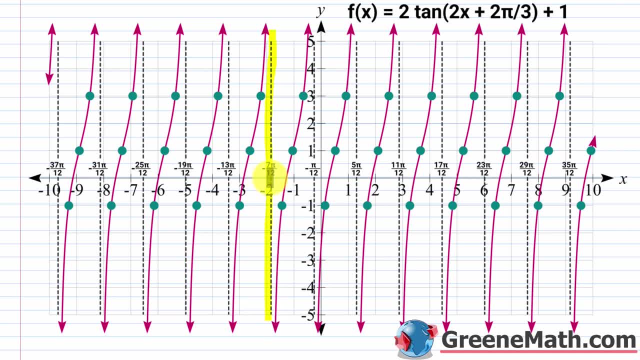 And this is the leftmost one that we found. So x equals negative 7 pi over 12.. Again, if you plug that in for x there, you're going to get undefined. So that's why you're getting a vertical asymptote there. Then this guy right here is going to be our. x equals negative pi over. 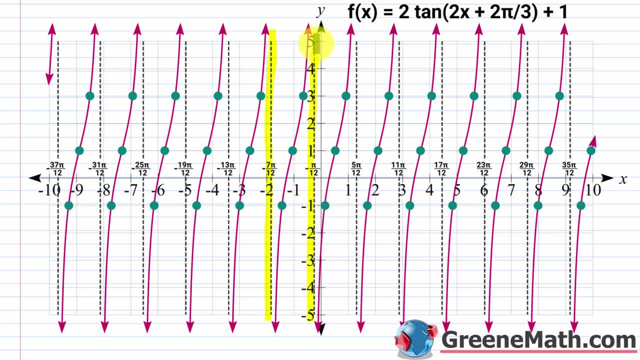 12.. Again, if you plug that in for x, there you're going to get undefined. So you're getting this vertical asymptote here. Our next goal is to figure out what is this point, this point and this point? So this is the quarter of the way through, this is halfway or midway and this is 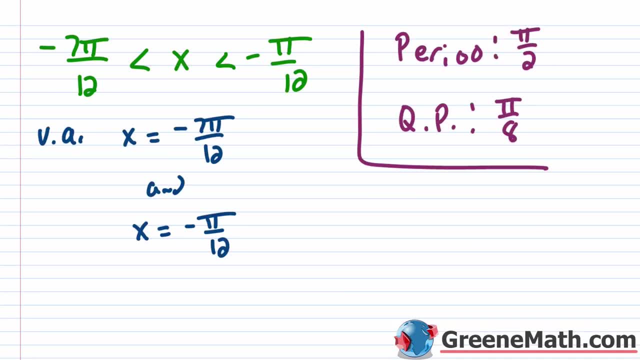 the way through. So let me come back And let's think about how we can use this information. So the first thing is you can find your x values by just adding quarter periods. So you can start with this: one x equals negative 7 pi over 12, add the quarter period of pi over 8. And you just 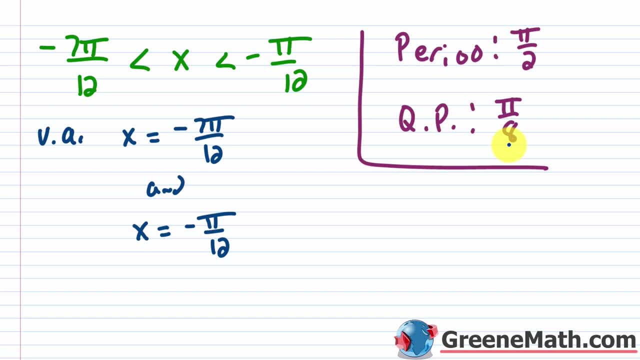 keep doing that to get the next x value and the next x value, the next x value, the y values you can either plug into the function or you can use graphing transformations, So I'll show you both. Let me go ahead and grab this real quick. So you have negative 7 pi over 12, and then plus pi. 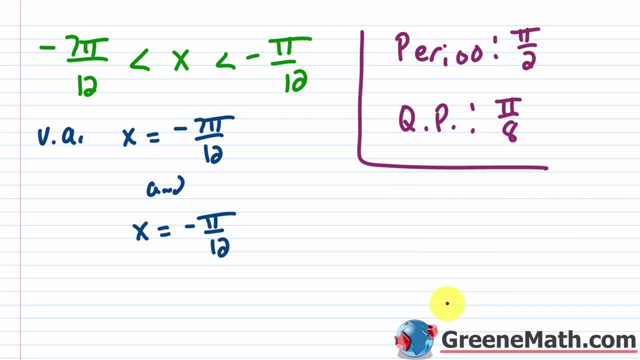 over 8.. I'm not going to have enough room to do this on the sheet, So I'm actually going to go to another page. If you're trying to find your x value for the first quarter point, let's multiply this by 3 over 3.. And let me slide this down. I'm going to multiply this by 2 over 2, just so we can. 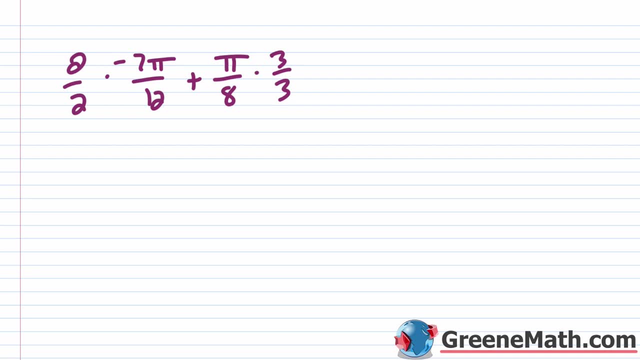 have a common denominator. If you notice, you have a denominator of 12 and a denominator of 8.. So this is basically 2 squared times 3.. And this right here is 2 cubed. So basically the LCD is going to be 24.. It's going to be 8 times 3.. So this right here would turn into: 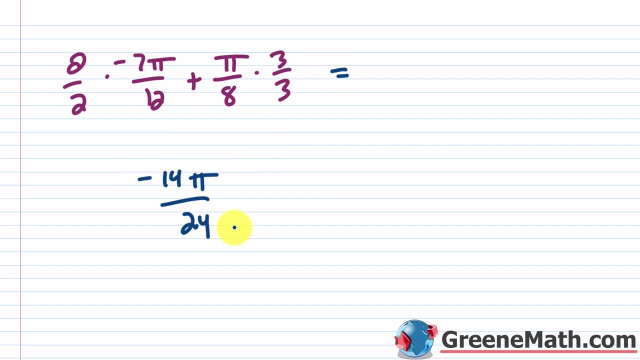 negative 14 pi over 24,. just multiplying 2 times negative 7 pi, that's negative 14 pi, And then 2 times 12 is 24.. And then, plus over here, 3 times pi is 3 pi, And this is over 8 times 3,. 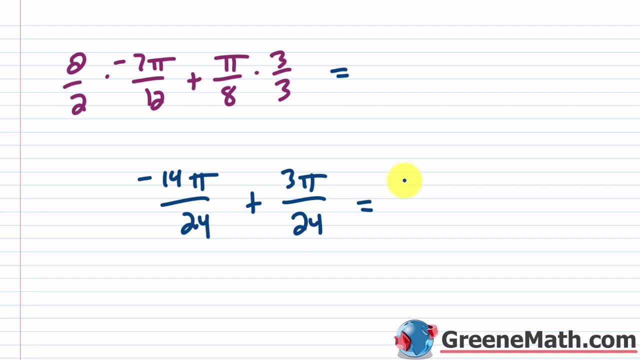 that's 24.. So if you do this, negative 14 pi plus 3 pi- that's negative 11 pi And this is over 24.. Okay, let me write this right here. So for my first quarter point, the x value is negative 11 pi. 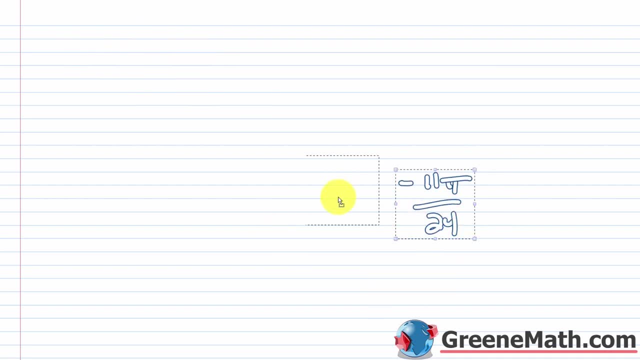 over 24.. The quarter period I listed as pi over 8. But again we could see that we could write that as 3 pi over 24. So we have a common denominator. So go ahead and add here: So negative 11 pi over 24, plus 3 pi over. 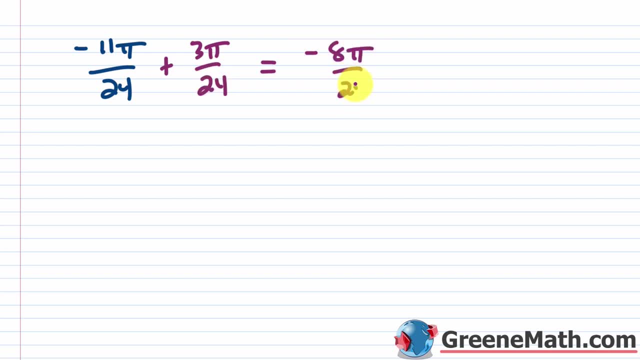 24,. that would be negative 8 pi over 24.. You can simplify that, but I wouldn't do it yet. Let's come down here. So this is for the halfway or midway. So basically, this is going to be negative. 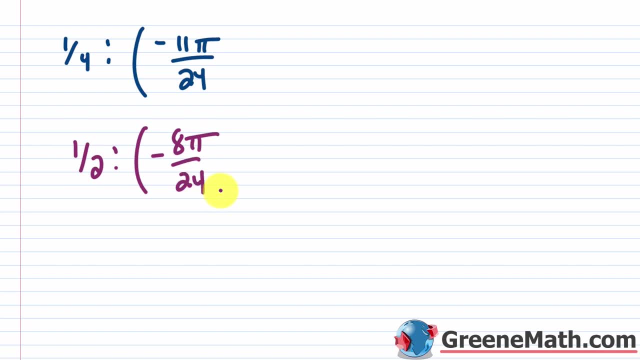 8 pi over 24.. And if you simplify that, 24 divided by 8, that would be negative 8 pi over 24.. 8 is going to be 3. And 8 divided by 8 is 1.. So this becomes negative pi over 3.. Okay. 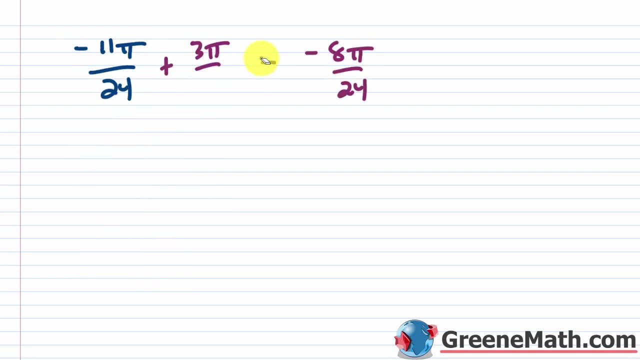 then we want our three quarters of the waypoint. So start with this And again just add a quarter period. So this is plus 3 pi over 24.. And let me slide this down over here. So this should be negative 5 pi over 24.. Just doing negative 8 pi plus 3 pi, that's negative 5 pi over the common. 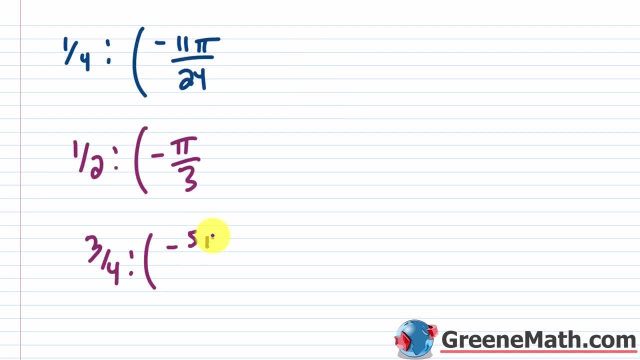 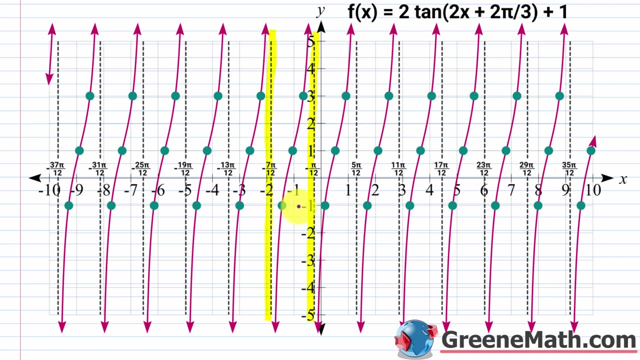 denominator of 24.. So negative 5 pi over 24.. So this is going to be negative 8 pi over 24.. And coming to the graph, we can see that for the first quarter point the y value is going to be: 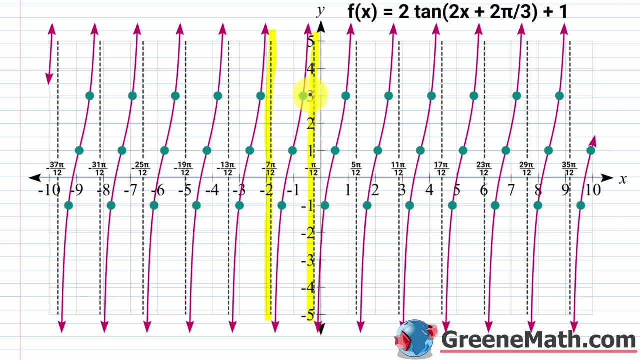 negative: 1.. For the halfway point, it's going to be positive: 1. And then, for the three quarters of the waypoint, it's going to be 3.. Now, how could we get that? Well, essentially, you could plug. 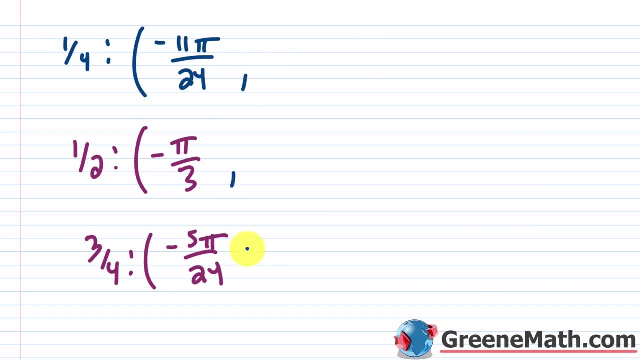 into the function or you could use graphing transformations. Let me just show you with this one right here that you could do it that way, And then I'll do the graphing transformations because it's a little bit faster. So, coming back up here, you would want to say what is f of negative 11 pi? 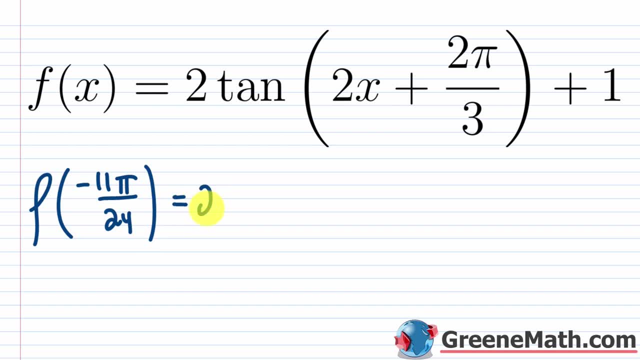 over 24.. So you're just plugging in. So this equals 2 times the tangent of. you have 2 times negative 11 pi over 24.. You're just plugging this right here in for x, right there. So that's all. 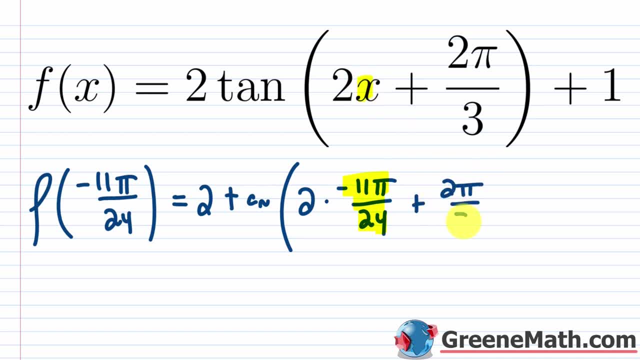 you're doing, And then we'd say plus 2, pi over 3, and then plus 1.. You can think about this canceling with this and giving me a 12 down here, And then I could multiply this. Let me scooch this. 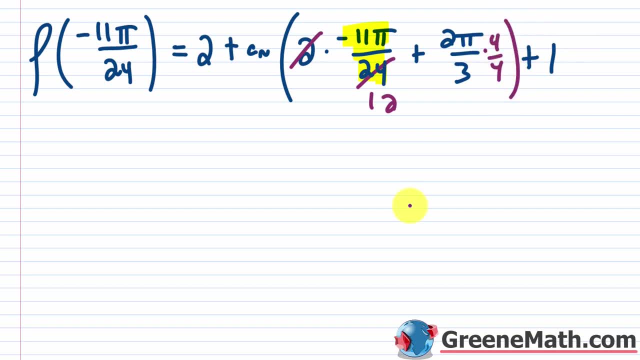 down a little bit. I can multiply this by 4 over 4. So I have a common denominator. So this would be negative 11 pi over 12. And then plus this would be 8 pi over 12.. So let me write that in. 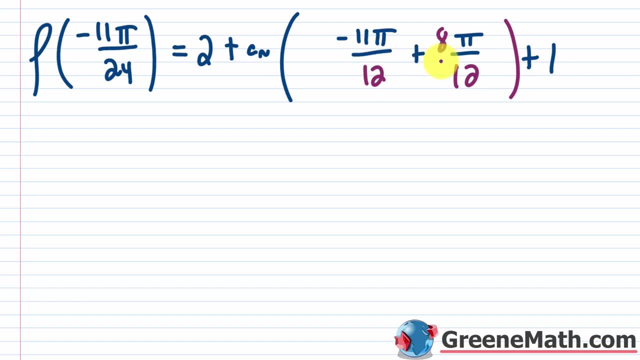 And then you would have negative 11 pi plus 8 pi. That's negative 3 pi. So you'd have negative 3 pi over 12.. Negative 3 pi over 12. And of course that's going to simplify to negative pi over 4.. 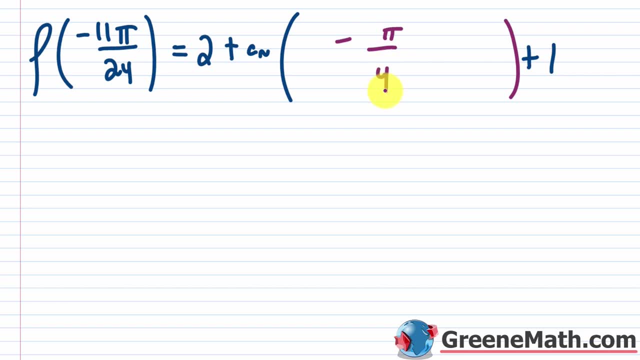 So negative pi over 4.. We know that the tangent of negative pi over 4 is negative 1.. So basically this becomes 2 times negative, 1. And then plus 1.. So 2 times negative 1 is negative 2. And then negative 2 plus 1 is negative 1.. 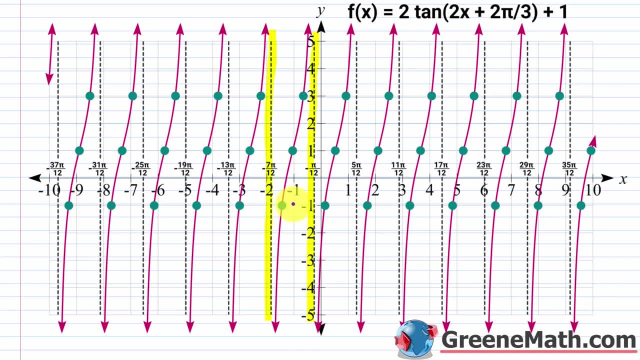 So this equals negative 1.. Again, if you go to the graph, you can clearly see the y-coordinate here is negative 1.. So let me put negative 1 in right there. Now, what's the other way to do this? 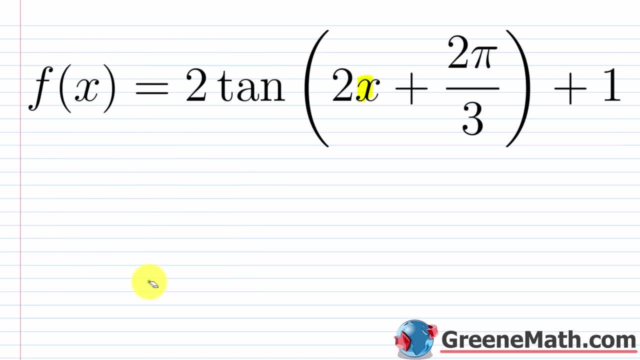 Because that's pretty slow. Well, you could have used graphing transformations. In other words, you know that on, y equals the tangent of x. you have these points which are for the quarter of the way through. Again, it's negative: 1 pi over 12.. So you could have used graphing transformations. 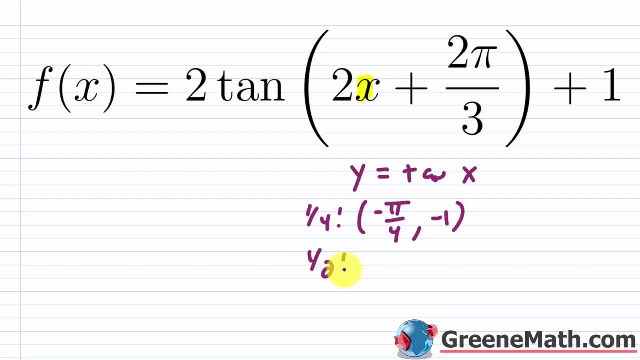 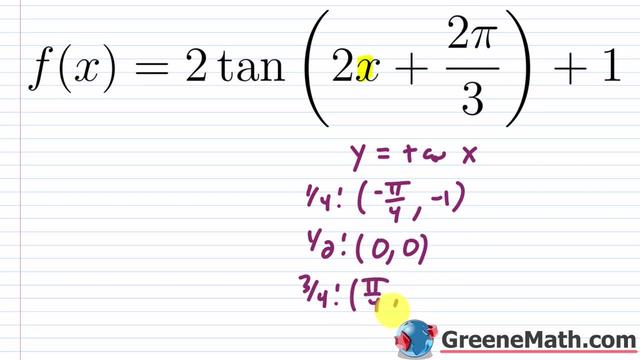 And then for halfway through it's going to be 0 comma 0. That's your x-intercept. And then for three quarters of the way, you're going to have pi over 4 comma 1.. Well, what's happening in terms? 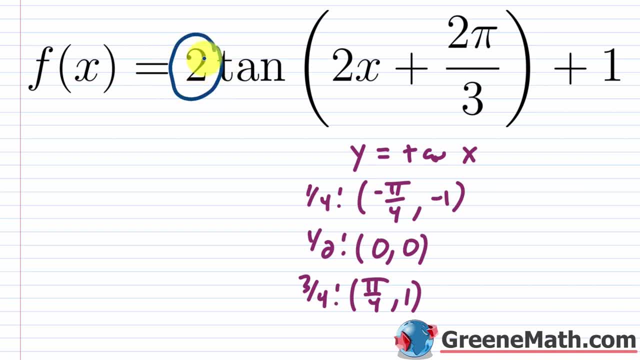 of the vertical transformations. Well, you have this 2 out in front, That's giving me a vertical stretch by a factor of 2. And then you have this plus 1 right here, which is going to give me a shift up by 1.. This is done first and this is done second. So, in other words, if I take this, 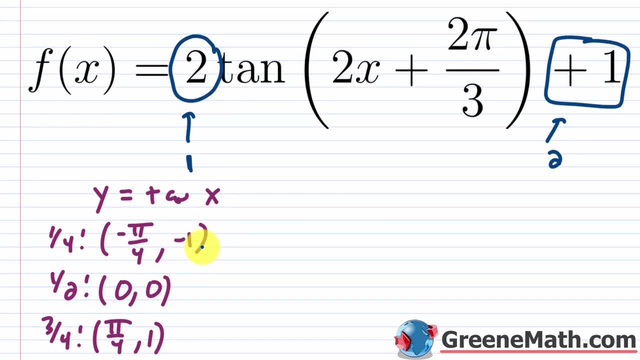 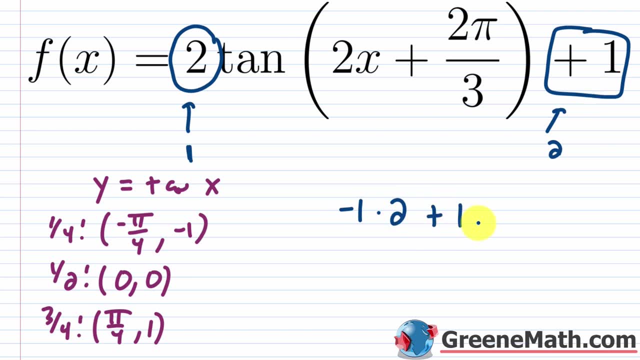 let me move this down here a little bit so it fits. So if I take this right here, this y-coordinate of negative 1, and I multiply by 2 first, and then I add 1 second, well, that's negative 1 times 2.. That's negative 2.. And then negative 2 plus 1,, that's negative 1.. 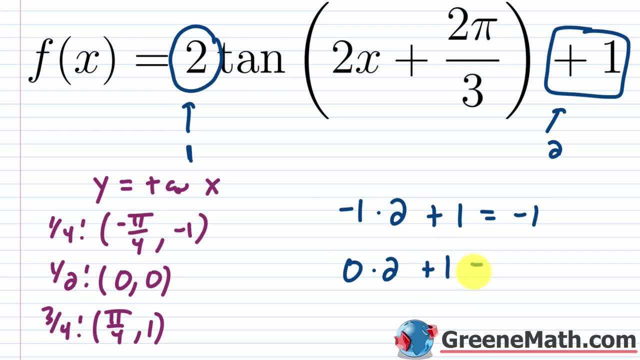 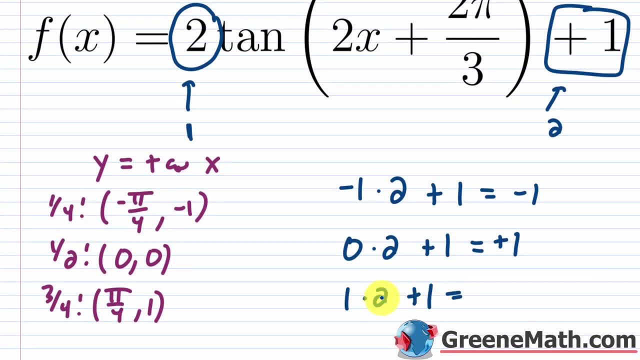 If I go through this one and I go 0 times 2 plus 1,, well, 0 times 2 is 0, plus 1 is 1, positive 1.. And then if I look at this one, I have 1 times 2 plus 1. So 1 times 2 is 2.. 2 plus 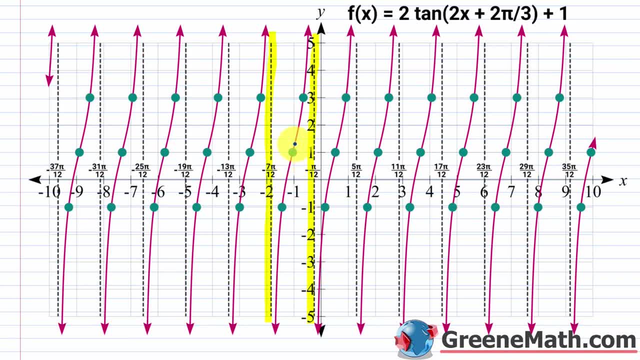 1 is going to be 3.. And that's exactly what we saw. If you look at for the halfway point, well, basically the y-coordinate is 1.. If you look at the three-quarters of the waypoint, the y-coordinate is 3.. Once you know those y-coordinates, when you go to the right or to 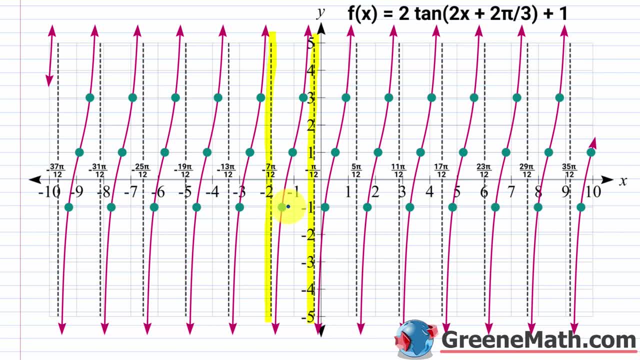 the left to extend the graph. those are always going to be the same. So for the first quarter point, it's always going to be negative. 1. For the halfway point, it's always going to be positive. 1. For the three-quarters of the waypoint, it's always going to be positive. 3. So you only need 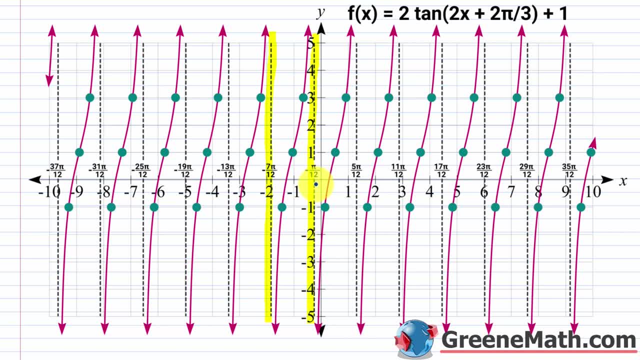 to figure out the x-coordinates for the vertical asymptotes and for the points that you're getting, And you can just do that by continually adding quarter periods. In other words, in terms of getting the x-values, you could start here: add a quarter period, add a quarter period. 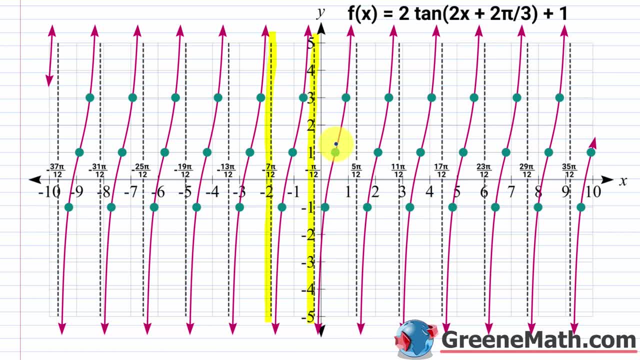 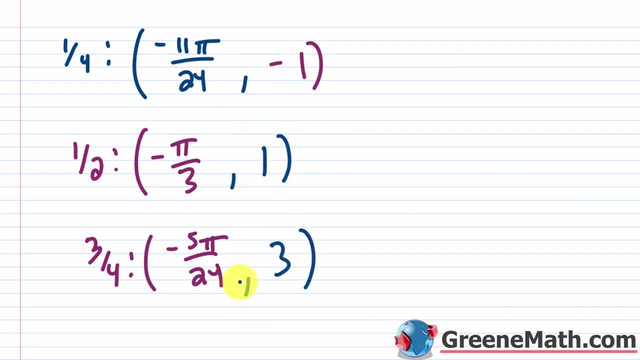 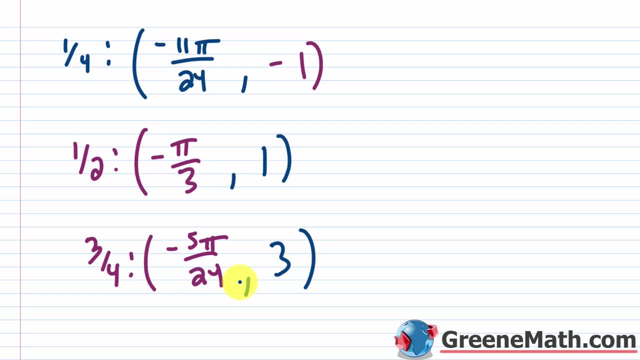 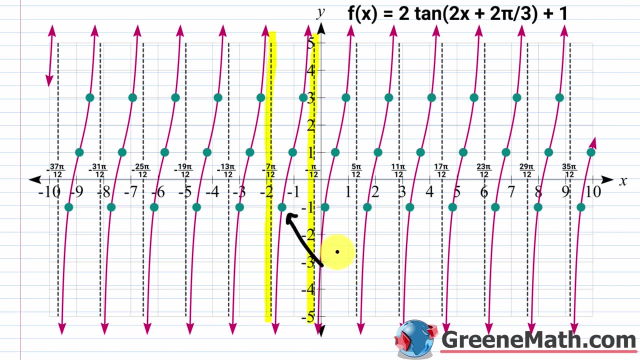 to you. I left you a very detailed graph on Desmos where all the points are filled in. But basically I can come through here and try to fill this in. It's going to be really tight, This point right here. let me just arrow to it and say it's negative. 11 pi. 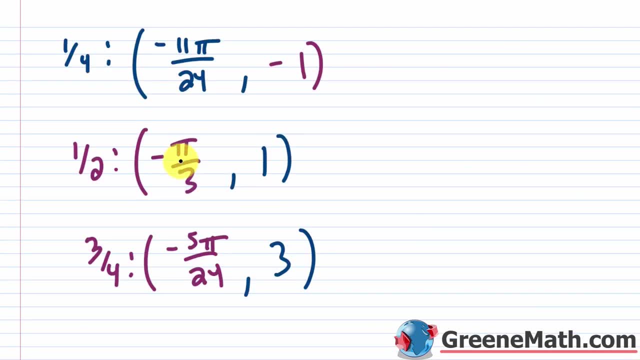 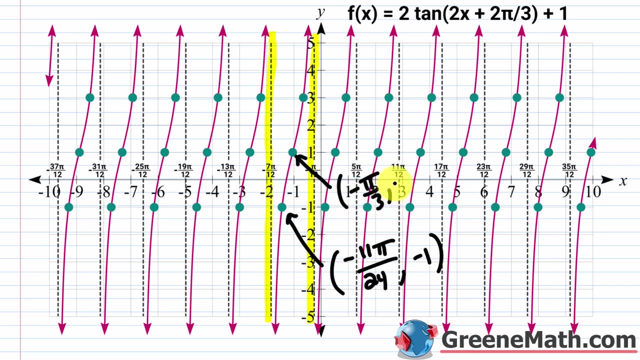 Over 24 and then comma negative: 1. Then you have your negative pi over 3 comma 1. So this right here is negative pi over 3 comma, positive 1. And then this one right here is negative: 5 pi over 24. 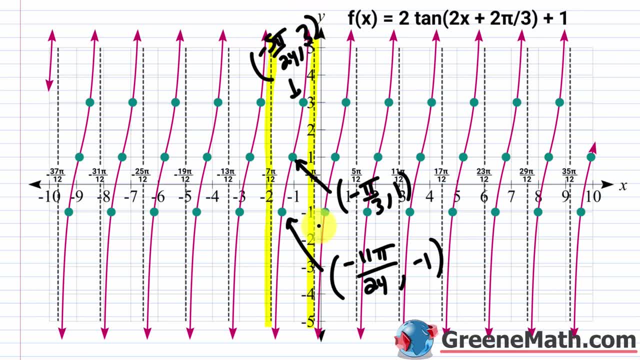 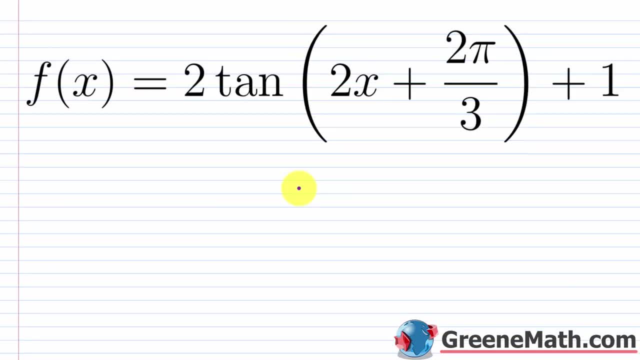 comma 3.. So, again, you can click that link and go to Desmos and see all of these points. I've labeled them for you. if you want to get more detail, All right. before I move on to the next problem, I want to show you this using only graphing transformations. This is something. 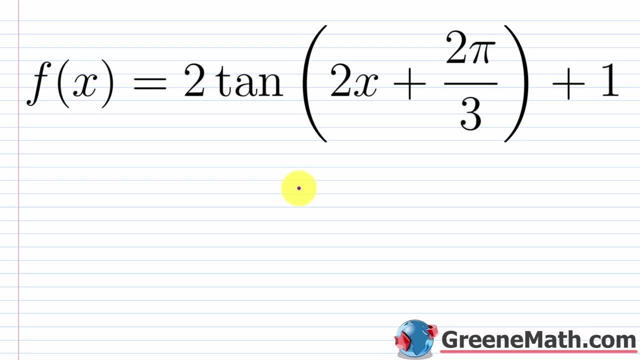 you should be aware of. In some cases it's faster, You may prefer to do it this way, But generally speaking it's very error prone because a lot of students have trouble with horizontal transformations, So things that affect the x coordinate. So let's just look at f of x equals. 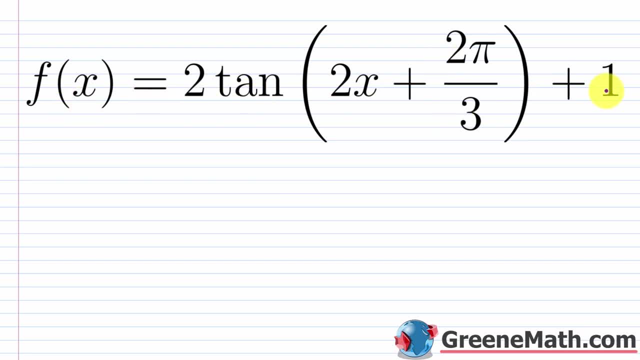 2 tangent of 2x plus 2 pi over 3 and then plus 1 and compare it to your f of x is equal to your tangent of x. So with this one, let me actually grab this real quick And let me come down here. 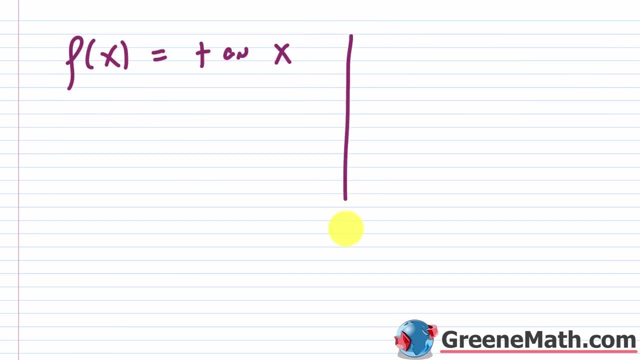 a little bit. You have your basic points, which we already know. at this point Let me put a little border here. The first quarter, So basically that's going to be negative pi over 4 comma negative 1. You have your halfway: that's going to be 0 comma 0. And then you have your three. 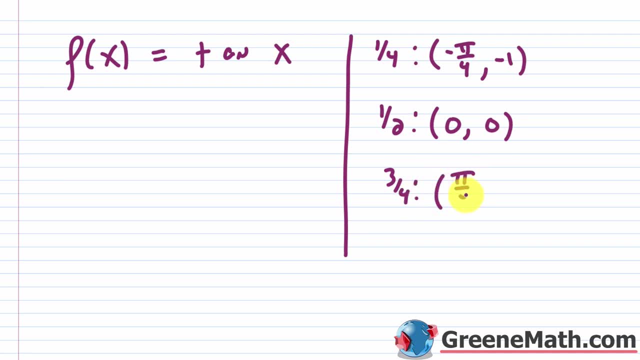 quarters, And basically that's going to be pi over 4 comma 1.. So you think about the transformation. So you're going to have a new x coordinate and a new y coordinate. Of course you also have the asymptotes to consider. So for that you just have to think about the x, So you'd have the 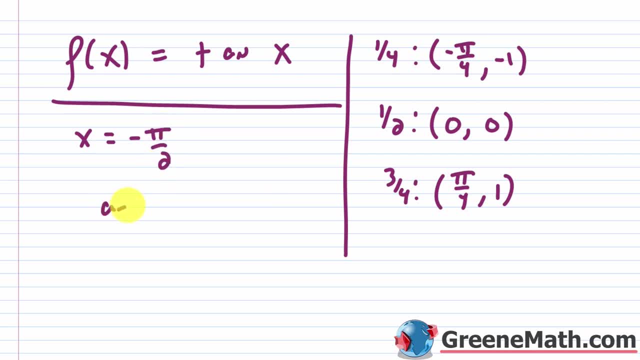 x is equal to negative pi over 2.. And so you'd have: x is equal to pi over 2.. And these right here, these are the vertical asymptotes. So let's come back up, And the first thing I would do is I would: 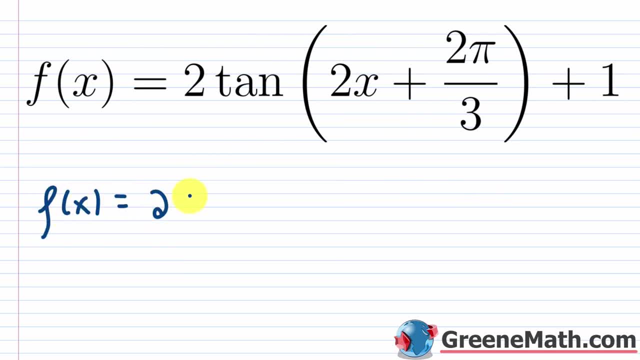 factor this, So I would say f of x is equal to 2 times the tangent of Pull out that 2 there. It's just going to make the phase shift a lot easier to find. So pull that out And then you're going. 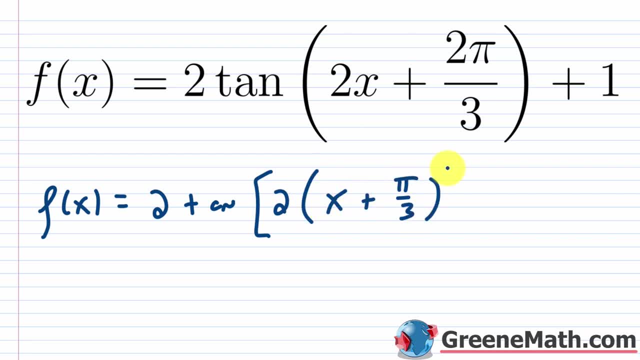 to have x plus pi over 3. And basically close that down and say this is plus 1.. I always like to check this. So 2 times x is 2x, And then plus 2 times pi over 3 is 2 pi over 3.. 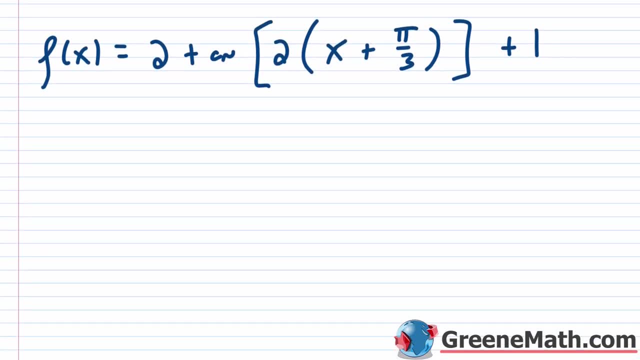 So that's good to go. So here is where it starts to get a little bit confusing. You have transformations that are happening to the y- Those are the vertical transformations- And you have transformations that are happening to the x- Those are the horizontal transformations. 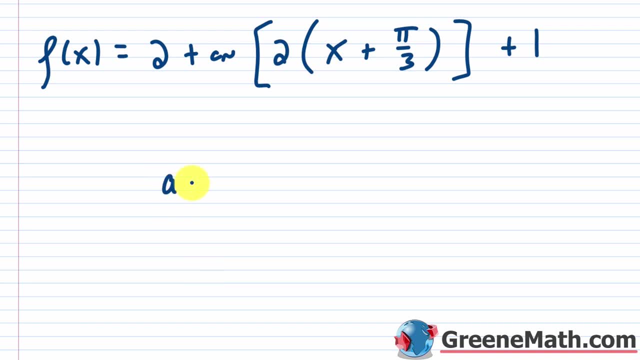 The vertical transformations are very straightforward. If you have something like a times, let's say f of x plus b, So let's say g of x is equal to this. So this is going to be a vertical stretch. And if you have a vertical compression, 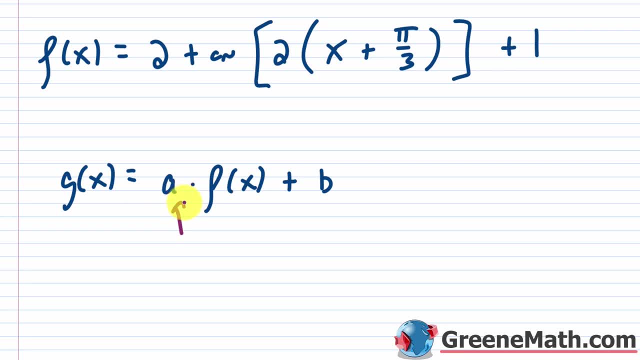 or sometimes you'll say a vertical shrink, if a is between 0 and 1.. Then for this one right here, this b: this is giving me a shift up if b is positive and a shift down if b is negative. So hopefully you know that already And in terms of the order, we follow just the order of 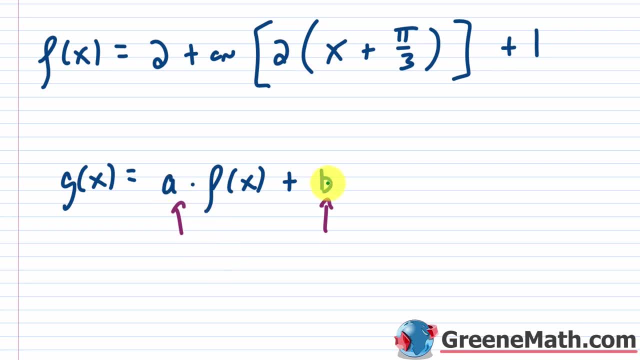 operations. You do multiplication before you do addition in the order of operations. So this is done first and this is done second, And then you have a shift up if b is positive And then you have a shift down if b is negative, And then you have a shift down if b is positive, And then you 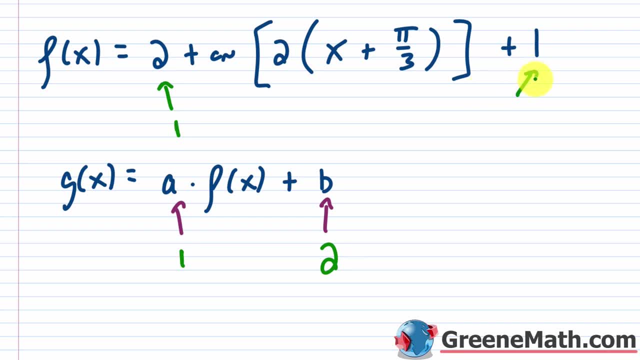 have a shift down if b is negative, And then you have a shift down if b is positive, And then you. So if I look at this, this is done first And this is done second. So we know that for the y coordinates- again we saw this earlier- you're going to multiply by two first, and then you're. 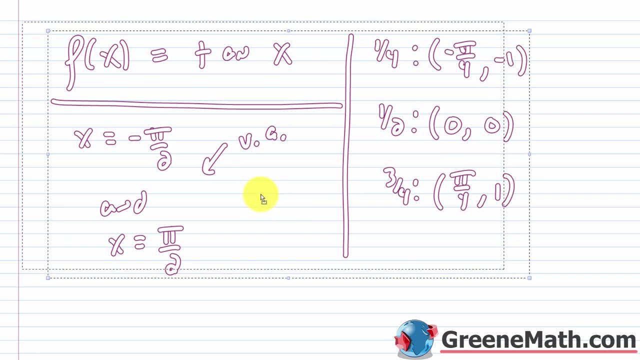 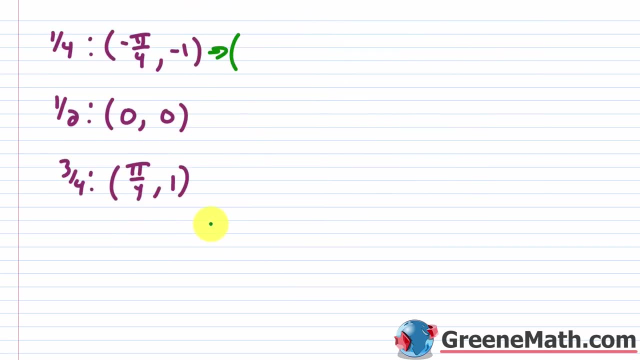 going to add one. So if we think about those points- and let me slide this over so this fits, when I go over here and I do my transformation, actually let me move this to another page because I don't think it's going to fit the way that it is. Basically, you can get the y values. 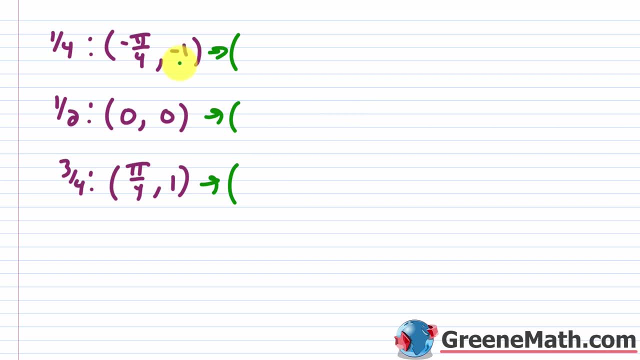 again. you multiply by two. first, So negative one times two is negative two. then you add one, So negative 2 plus 1 is negative 1.. And then for this: one 0 times 2 is still 0. Then you add 1,. 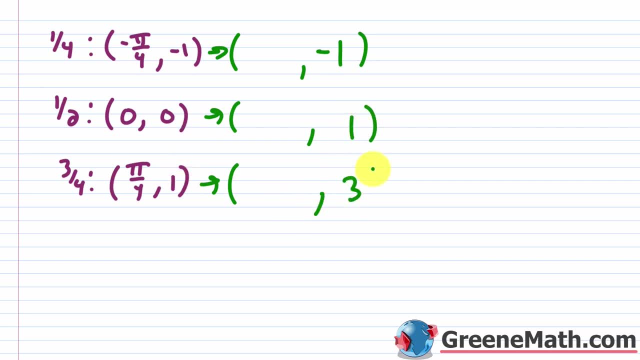 so that's 1.. And then for this one, 1 times 2 is 2 plus 1, so that's 3.. So that's very straightforward. It's done almost instantly. Now let's come up and let's think about the harder. 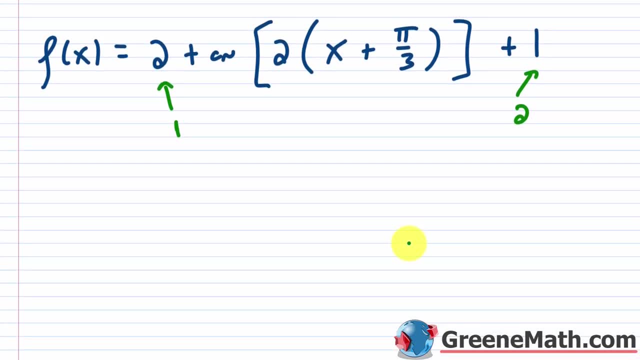 guy which is going to be what's happening to the x coordinates. Basically, what are the horizontal transformations? We know that if we have something like, let's say, g of x is equal to f of, let's go ax here, this is going to be: if a is greater than 1, you have a horizontal 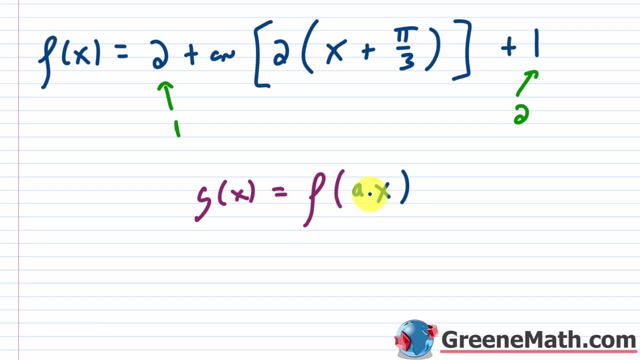 compression, or you could say a horizontal shrink, And then if a is between 0 and 1, now you're going to have that horizontal stretch. So it's always the opposite of what you think. So basically here, when you think about that 2, well that's something that's greater than 1.. So that is. 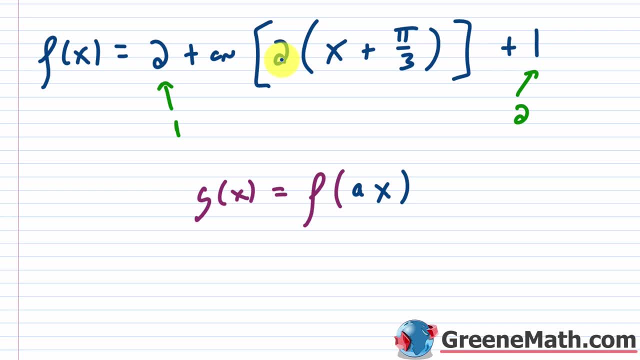 going to give me a horizontal compression, or you could say a horizontal shrink. however, you want to say that. Now, this is the confusing part, because there's different terminology. Some people will say that there's a horizontal compression by a factor of 2. If you want to say that, that's fine, Typically, 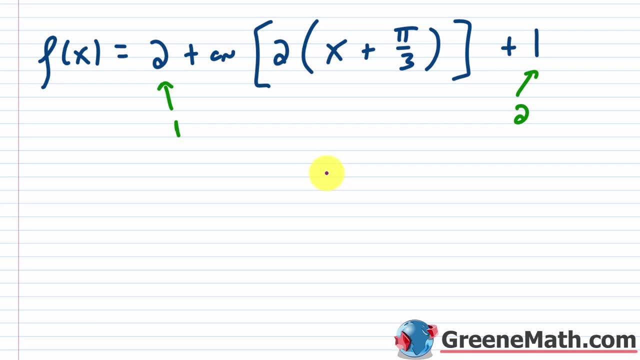 I'll say it that way. Other people will say that it's been horizontally shrunk by a factor of 1- half. Whatever you want to use in terms of the terminology, just realize that you're going to either be dividing by 2 or multiplying by half. Whatever you want to do there and whatever you, 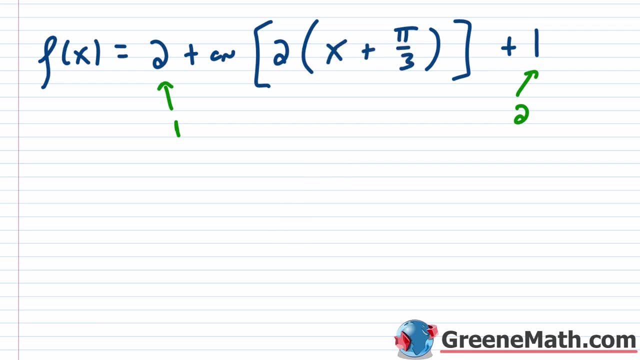 want to say: just realize what's happening Now. this part, right here, this is your phase shift. And again, it's the opposite of what you think. If you have x plus pi over 3, that means that I want to go pi over 3. 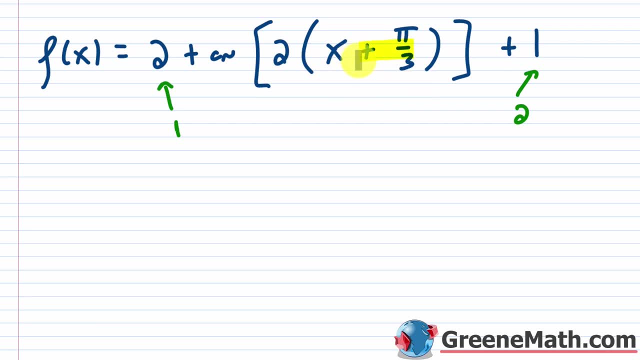 units to the left. I want to go minus pi over 3.. It's always the opposite of what you see. So what you would want to do here is actually do this one first and then this one second. So why is that the case? If we were to think about the order of operations, then you would want to do what's. 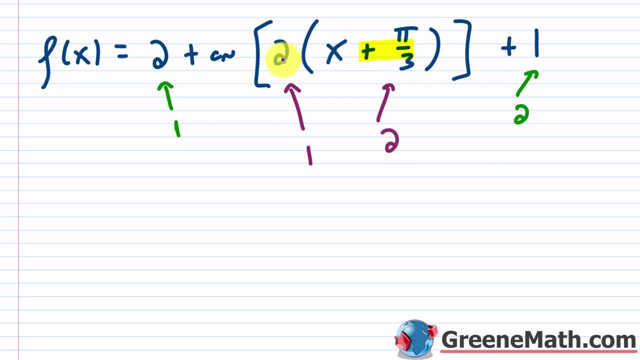 inside the parentheses first, and then what's outside, which in this case would be multiplication, second. But again on the inside, you have to reverse everything. This looks like it's going to be multiplied by 2.. Well, I have to do the opposite of that. I have to divide by 2.. This looks like I'm 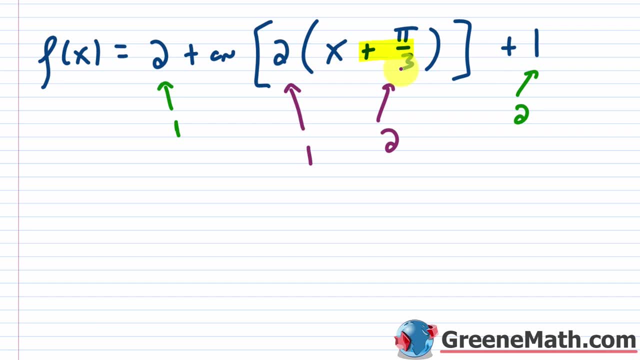 adding pi over 3.. I have to do the opposite of that, I have to subtract pi over 3.. And then the same thing happens with the order of operations. It has to go in reverse now. So basically it has to be this one first and then this one second. So if we think about all the x values, the first 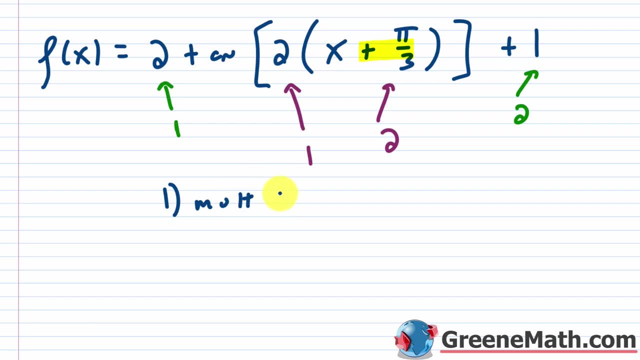 thing you're going to do is you're going to multiply by one half, Or again you could divide by 2.. And that's because you have to undo this part right here. You undo multiplication by 2 by dividing by 2 or multiplying by half. Then the second guy here that you're 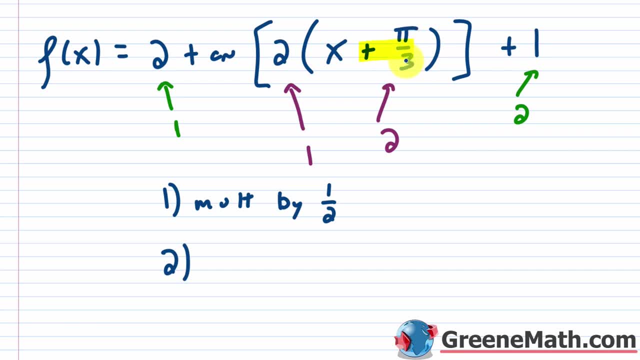 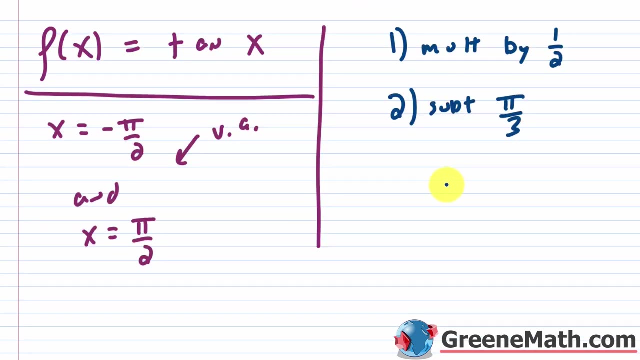 going to do? you're going to subtract away pi over 3.. So you can just write subtract pi over 3 or you could put add negative pi over 3.. So this is what we need to do to each x to get those x coordinates. So let me come down here. We'll do it through the asymptotes first. So if 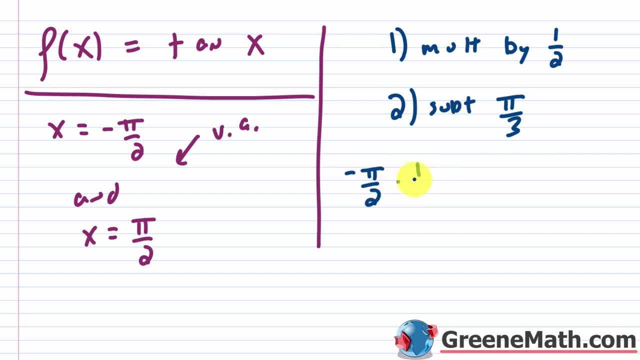 you start with negative pi over 2 and you multiply by one half. first that's going to be negative pi over 4.. And then, in step 2, you're going to take negative pi over 4.. You're going to need a common 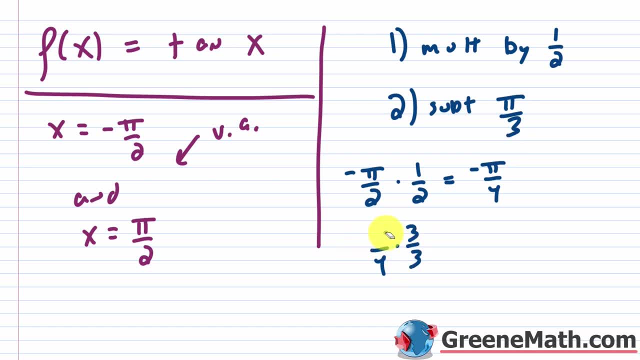 denominator. So let's multiply this by 3 over 3 now, So that would be negative 3 pi over 12.. So you can have negative 3 pi over 12. And you're going to subtract away pi over 3.. Let's write: 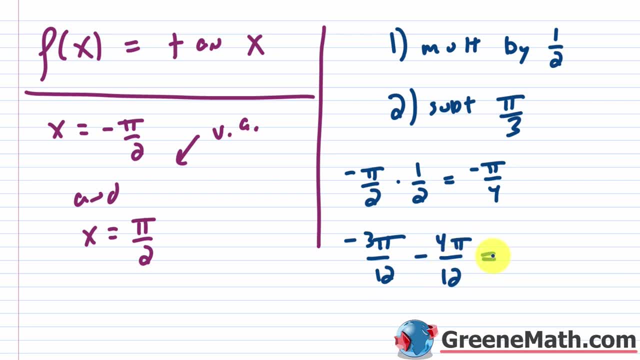 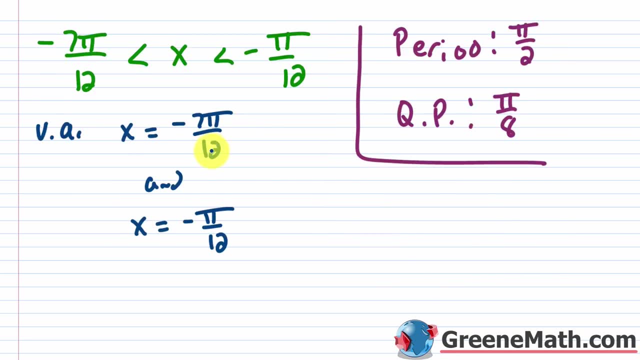 that as 4 pi over 12, just getting a common denominator. If you do the subtraction, you're going to get negative 7 pi over 12.. Notice that matches exactly what we got right here when we solve the problem in a different way. So you get x equals negative 7 pi over 12.. The other guys 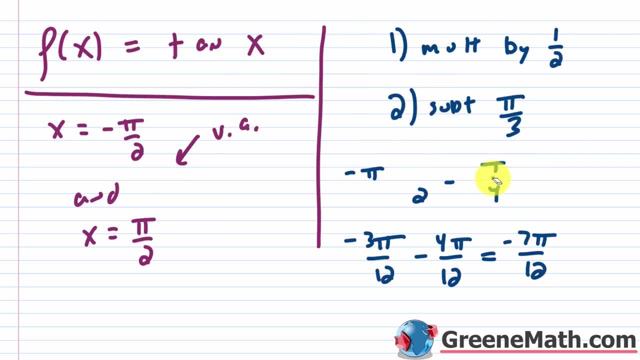 it's going to be: x equals negative pi over 12.. So let me erase this. And then, for this one again, all you're going to do, you're going to multiply by a half. So pi over 2 times a half. 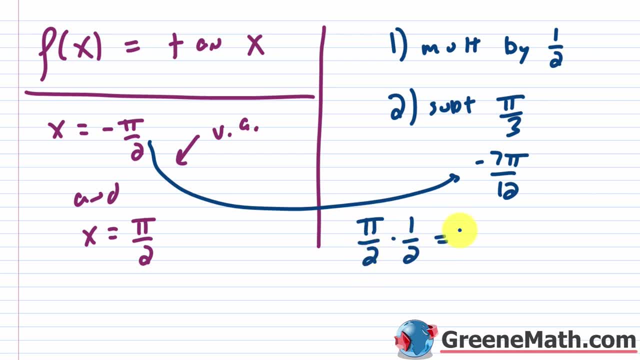 that would give me- let me actually show this- So pi over 2 times one half. this would be pi over 4.. So that's done first, And then, once you have that, you subtract away pi over 3.. So you: 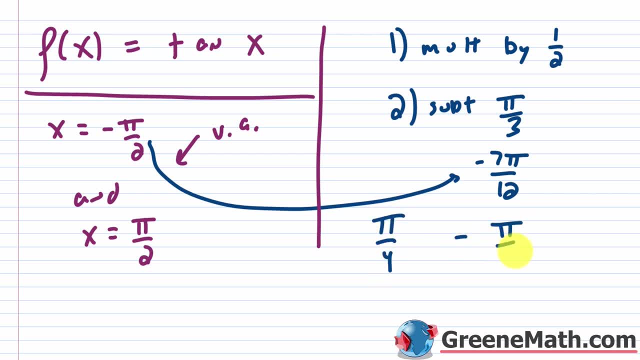 have pi over 4 and then minus pi over 3. Again, get a common denominator. This would be multiplied by 3 over 3. So this would be 3 pi over 3. And then, once you have that, you subtract away pi over. 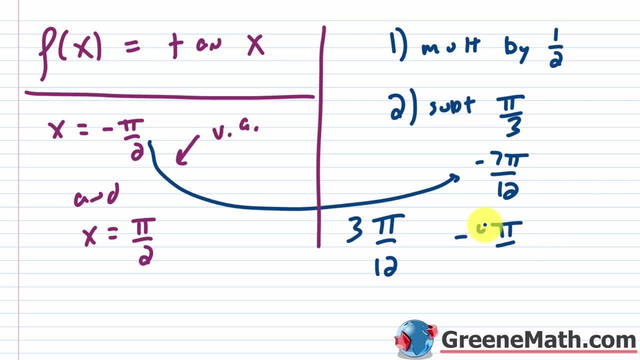 4 over 12.. Multiply this by 4 over 4.. So this would be 4 pi over 12.. So 3 pi minus 4 pi would be negative pi over the common denominator of 12. So negative pi over 12.. Again, as I just told you, 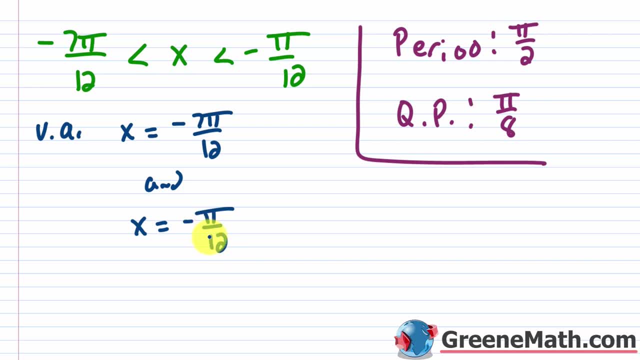 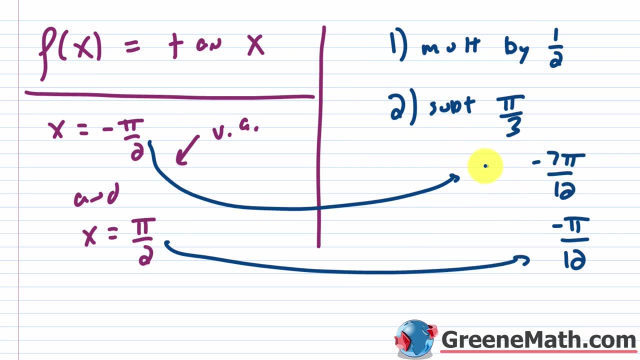 x equals negative pi over 12.. That's your other vertical asymptote that we found earlier using the other approach And we'll arrow to this. So the vertical asymptotes here for this guy you would have: x is equal to negative 7 pi over 12.. And then x is equal to- let me put and in: 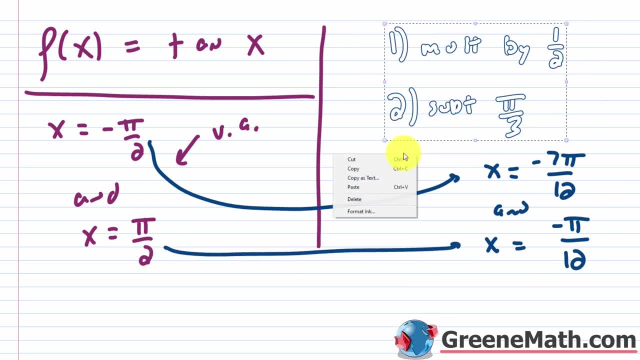 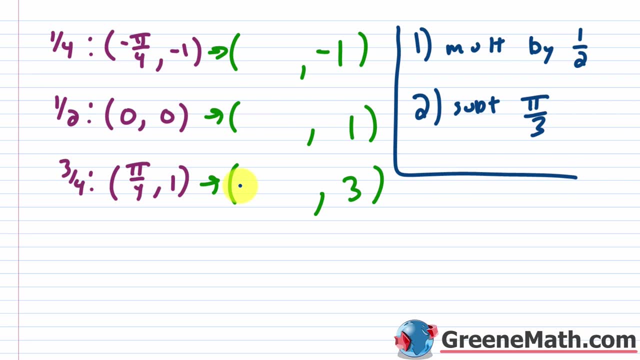 here. So that's how you could find that using the graphing transformations only. Let me go ahead and copy this real quick And let me come down here and paste this in: For getting the x coordinates for these three points again, you just follow the same procedure: Multiply by half, then subtract. 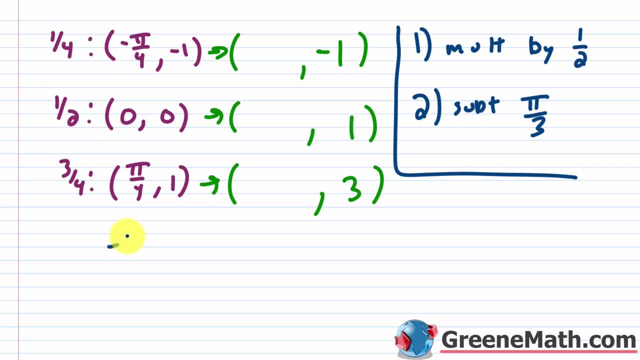 away pi over 3.. Negative pi over 4 times a half. negative pi over 4 times one half: That's going to be negative pi over 8.. So once you have that, you're then going to subtract away your pi over 3.. 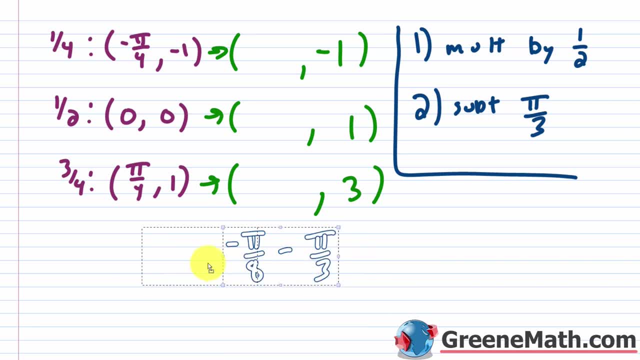 So minus pi over 3.. We need a common denominator. That's what makes it take so long. So let's say this is negative: 3 pi over 24.. Just multiplying this by 3 over 3.. And then minus. let's multiply this by 8 over 8. So 8 pi over 24.. And we get. 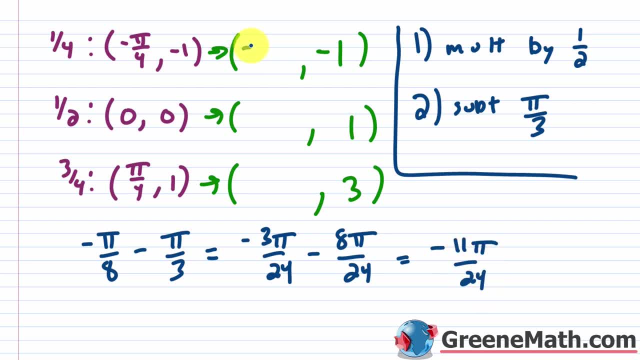 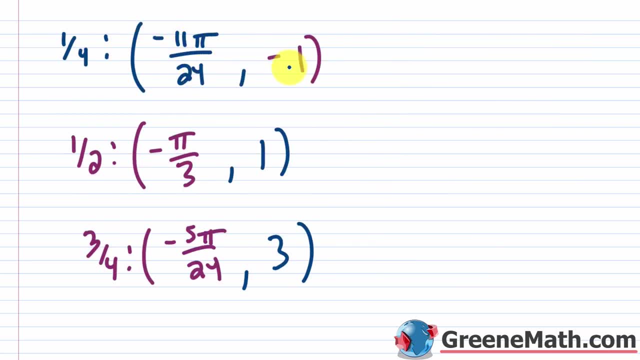 negative: 11 pi over 24.. And we know that's the case. So negative 11 pi over 24.. Again, if you check with what we did earlier, here's negative 11 pi over 24, comma: negative 1.. The next one's: 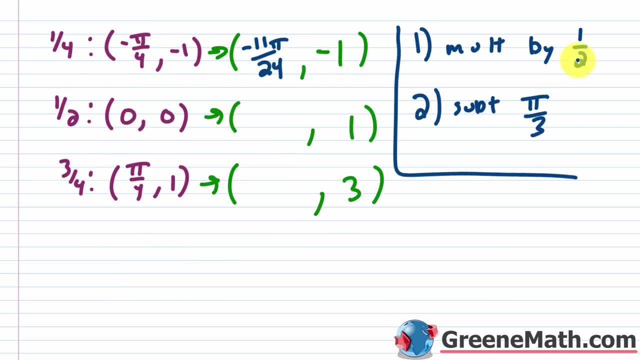 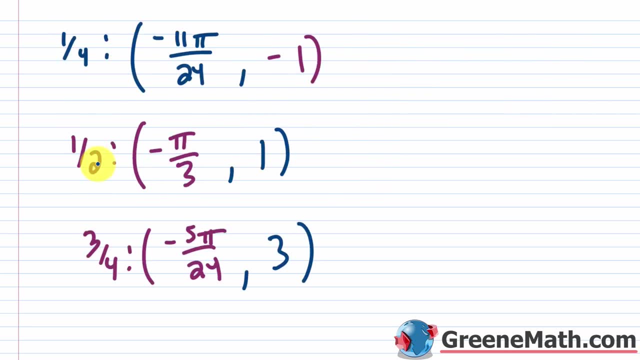 a little bit easier, because you're working with zero. So zero times a half is still zero. So then you just need to subtract away pi over 3. So this becomes negative pi over 3.. And so negative pi over 3, comma 1.. Again, here's your. 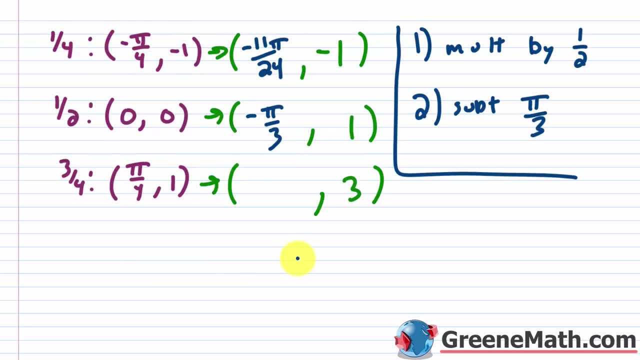 halfway point. So negative pi over 3, comma 1.. And then for the last one you have pi over 4 times one half. So that's done first. So this would be pi over 8. So then we have to subtract away pi over. 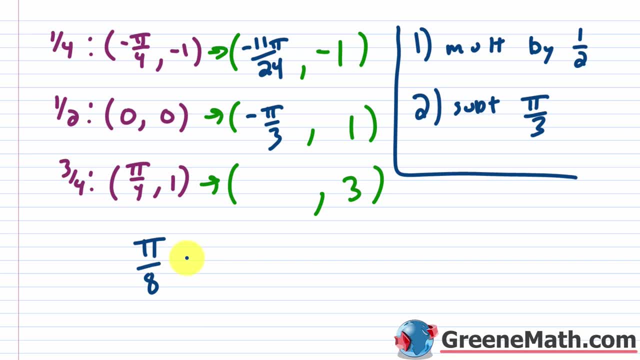 3 from that. So you have pi over 8. And then minus pi over 3.. Again, just get a common denominator. I'm going to multiply this by 3 over 3.. So this is 3 pi over 24.. And then minus you, multiply this. 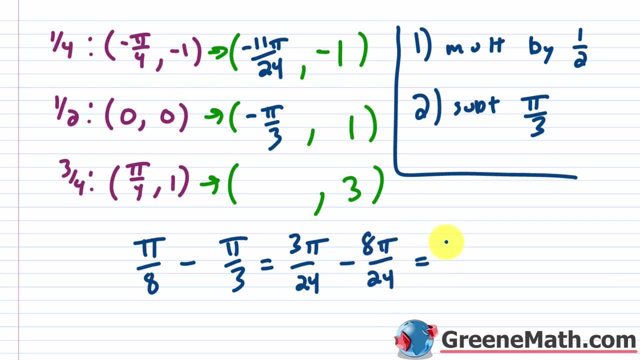 by 8.. So this is 8 pi over 24.. And this gives me negative 5 pi over 24.. So this is negative 5 pi. Let me make this 5 better here Over 24,, comma 3.. And let me show you that real quick. Here's: 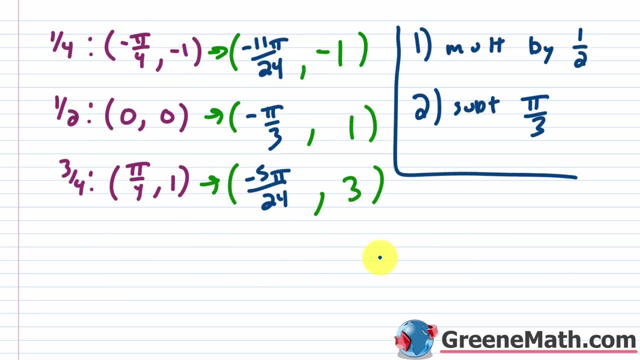 your negative 5 pi over 24, comma 3 that we found earlier. So of course you can use this approach. Many students like it because it's a little bit faster. But you really have to understand all the different graphing transformations, particularly what's being done to x and what. 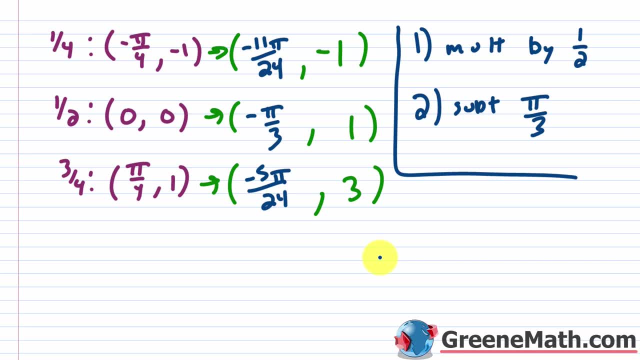 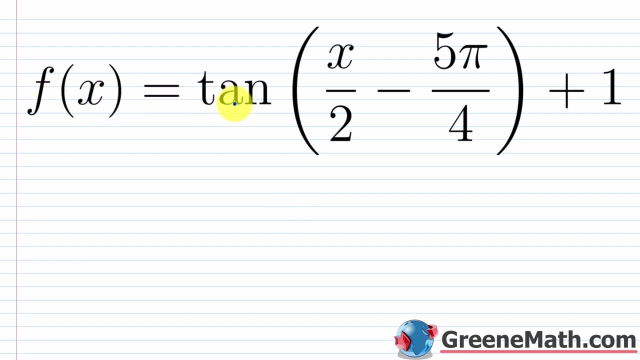 order. So if you have that down, then you could use this method. In some cases it's a little bit faster. All right, let's take a look at another example with tangent. So here we have: f of x equals the tangent of x over 2, minus 5, pi over 4, and then plus 1.. So again, you can use the book. 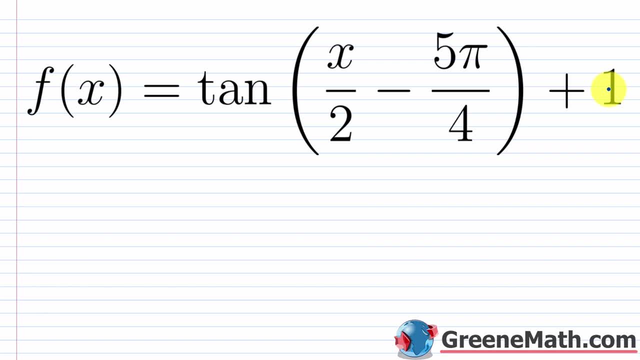 procedure, the one that I started out with, or you could use graphing transformations. It's really up to you. I'll do this one both ways again, And then, for the ones that we're going to do with cotangent, we'll have two examples. I'll just pretty much stick to the book method for 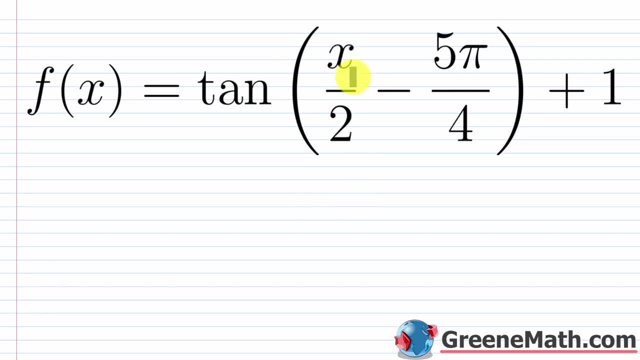 those. So let's start off with our book method. Again, you're going to take this right here, the argument for the tangent function, and you're going to say x over 2 minus 5 pi over 4.. And you're going to first say that this is greater than negative pi over 2 and less than pi over 2.. 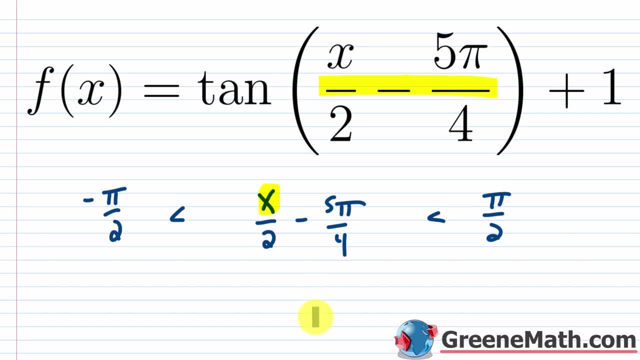 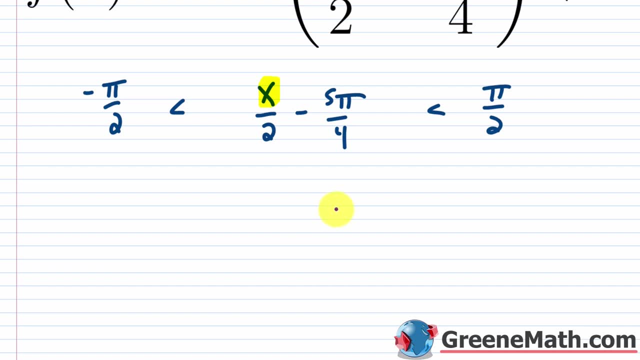 So your goal is to solve for x, So we want to solve for this guy right here. So what you could do again, if you have fractions involved, is just clear them first. It just makes your life a lot easier. And so what you see is you have a denominator of 2.. 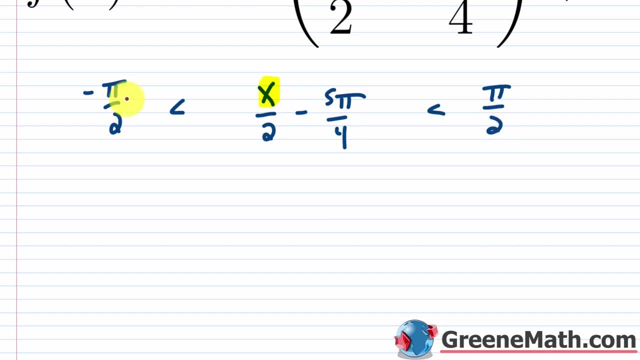 2,, 2,, 4, and 2.. So the least common denominator would be 4.. So just multiply everything by 4 here, And let me do that, like that and like that. So this 4 would cancel with this 2 and give me a. 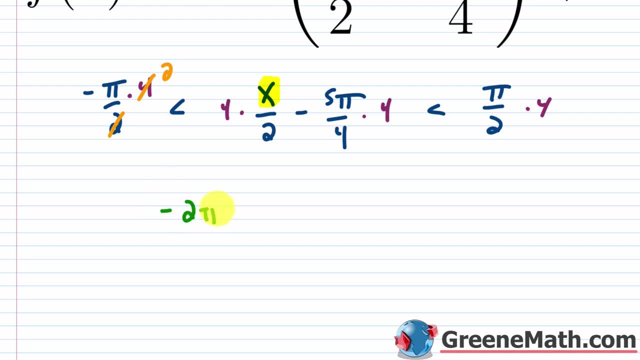 2. 2 times negative pi is negative 2 pi, So this is less than 4. would cancel with 2 and give me 2.. 2 times x is 2x And then minus these 4s would cancel, So you have 5 pi And this is less than. 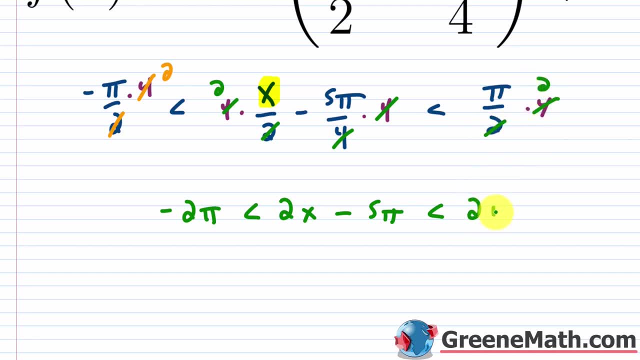 4 would cancel with 2 and give me 2.. 2 times pi is 2 pi Again. if I'm trying to solve for x, what do I do? Well, first I would add 5 pi to each part. So let's go ahead and do that, And let me move this. 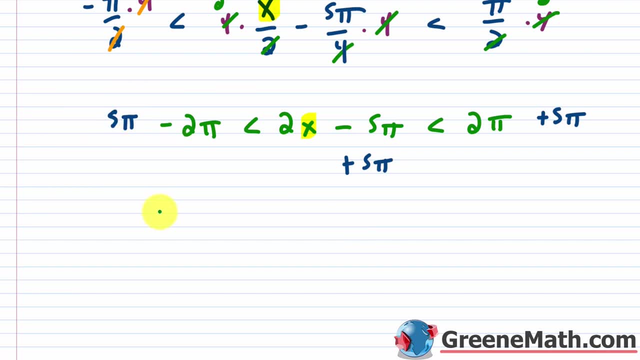 in a little bit more like that. So on the left, 5 pi minus 2 pi is going to be 3 pi, So this is less than 2x. Let me show this as canceling, which is less than 2 pi plus 5 pi. That's going to be. 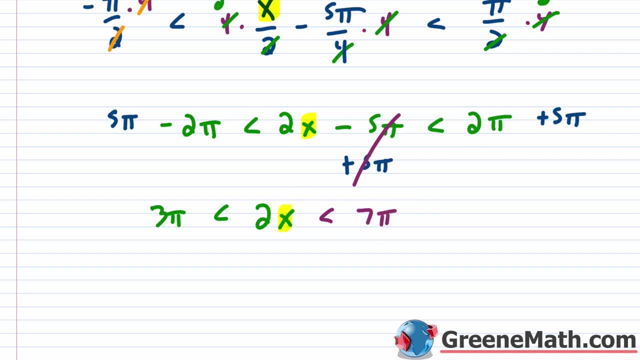 7 pi. Again, if you want to isolate x here, just divide each part by 2.. So let's go ahead and say: this is divided by 2,, this is divided by 2, and this is divided by 2.. 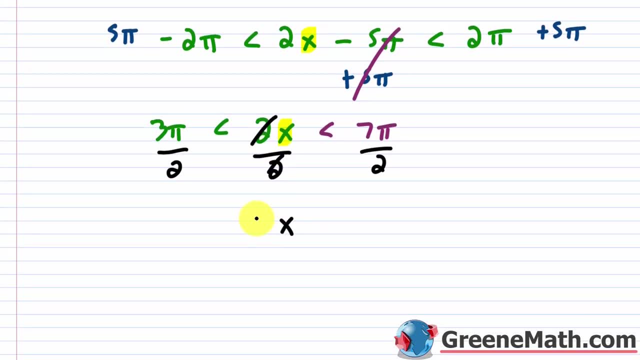 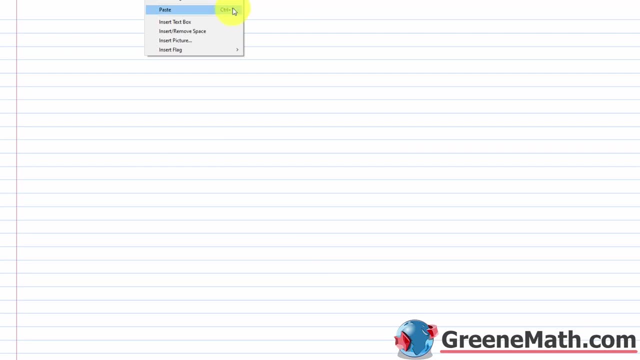 This would cancel. Let me slide down here a little bit. And so now we have: x is greater than 3 pi over 2 and less than 7 pi over 2.. And let me come down here to a fresh page. So again, just getting. 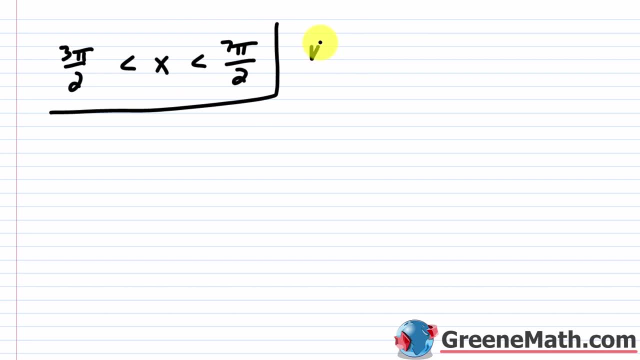 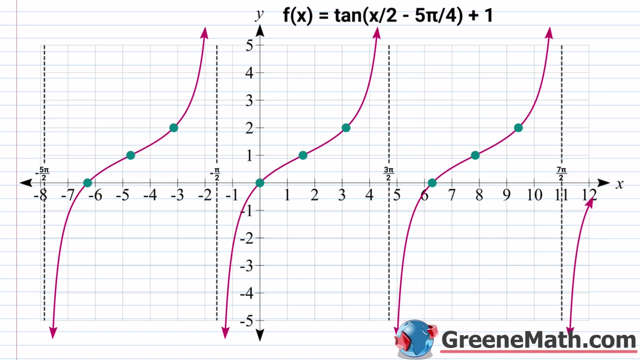 the information for the consecutive vertical asymptotes. So, vertical asymptotes: you're going to have x is equal to 3 pi over 2.. And then and you're going to have x is equal to 7 pi over 2.. So if you want to come to the graph again, I gave you a link for a more detailed version on Desmos. 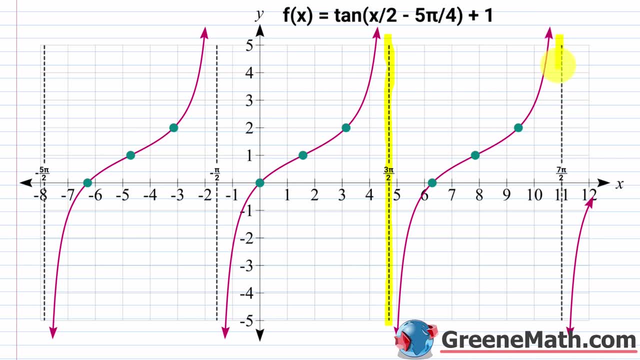 This is your x equals 3 pi over 2.. And then this is your x equals 7 pi over 2.. So so far we have that, But we need these three points Again. you're a quarter of the way, halfway, three quarters of. 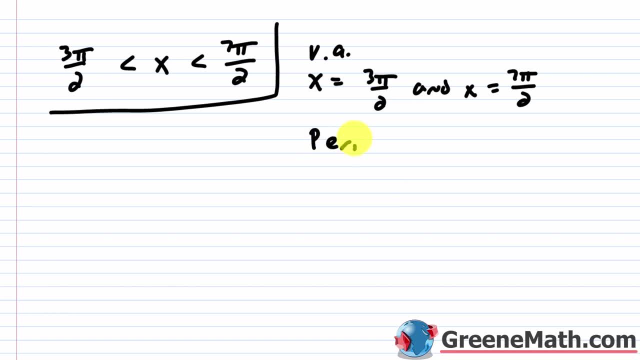 the way. The first thing is we do need the period. So what is the period? Let's go back up. So this right here is x over 2.. You could really write that as 1 half times x, So you could say this is: 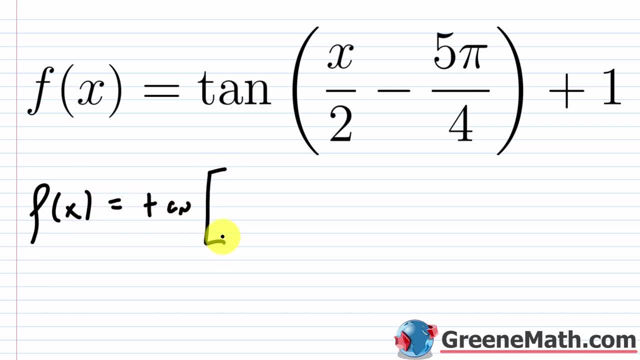 the tangent of- let me factor this, because we're going to do this with all graphing transformations in a little while, So that'll already be done. Let me pull out a 1 half, So inside you'd have x minus. So then, for this part right here, if you pull out a 1 half, it would be 5 pi over 2.. Close. 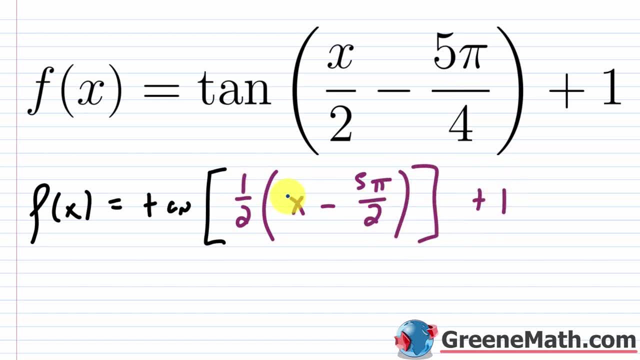 that down, close this down and then plus 1.. Again, if you want to check this, 1 half times x is 1 half x or x over 2. if you want to write it that way, Then you have minus and minus And then 1. 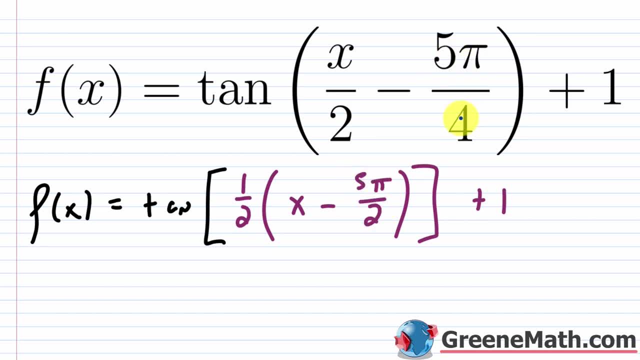 half times 5 pi over 2 would give me 5 pi over 4.. So that checks All right. So if we look at it now, you have this 1 half here, So the period is going to be pi divided by 1 half. So pi divided. 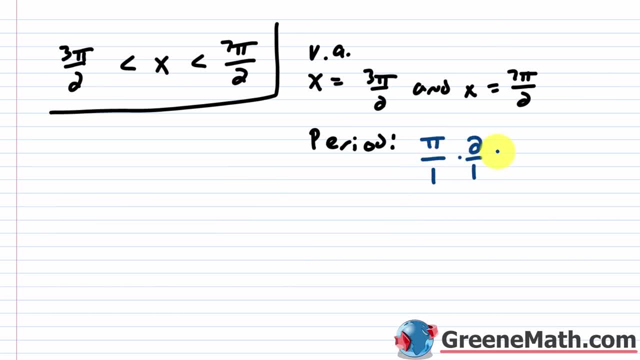 by 1 half, So you can go pi over 1 times 2 over 1, which is 2 pi. Okay, So now we know that the period is 2 pi And then the quarter period again. you just divide this by 4 or multiply it. 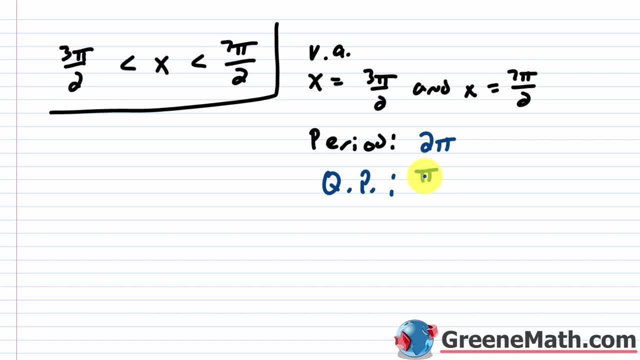 by a fourth. We know that 2 pi over 4 would be pi over 2.. That's your quarter period. So if you want to get your x values, you're going to start with this 3 pi over 2.. And then you're going to add quarter periods. Let me come down here. So let me start with 3 pi. 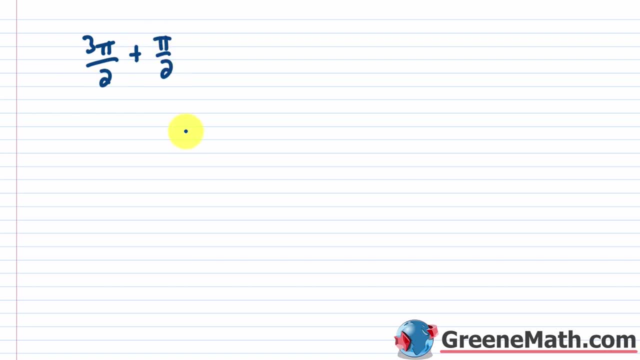 over 2.. And I'm going to add pi over 2.. And then basically that's going to give me 4 pi over 2.. So let me write this as the quarter point. So the first quarter you're going to have 4 pi over 2,. 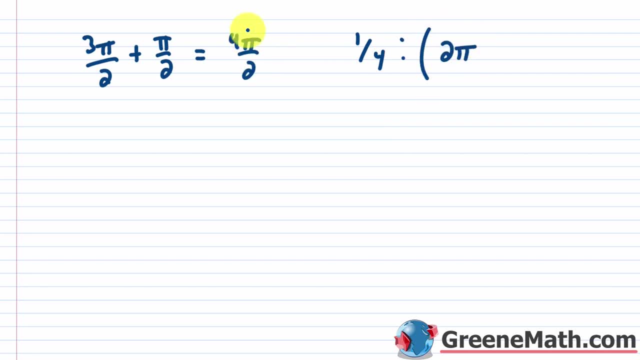 if you want to do that now is going to be 2 pi if you simplify, But keep it like this for adding. So for the next guy you're going to go 4 pi over 2 plus pi over 2.. That way you don't have to worry. 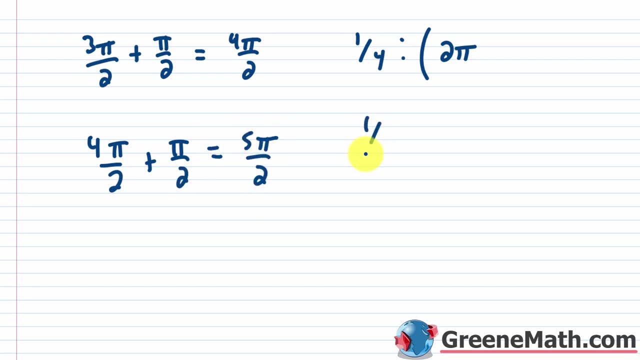 about the common denominator. This will give me 5 pi over 2.. So for the halfway point or the midway, as a lot of books say, you have 5 pi over 2 for the x coordinate. And then we'll do this one more. 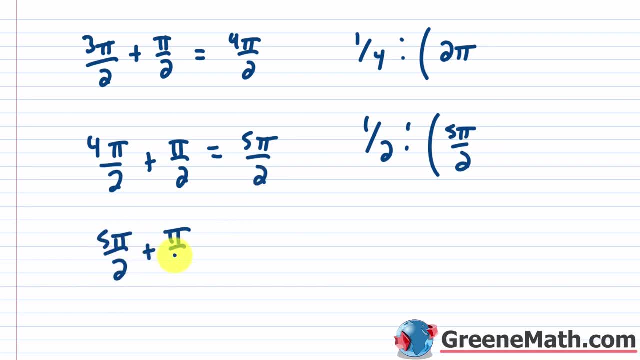 time. So 5 pi over 2, and then plus pi over 2.. This is going to be 6 pi over 2, which of course is 3 pi. So let's say that this is the three quarters point And basically the x value there. 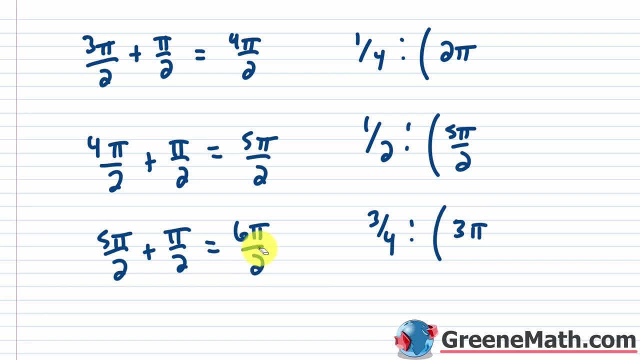 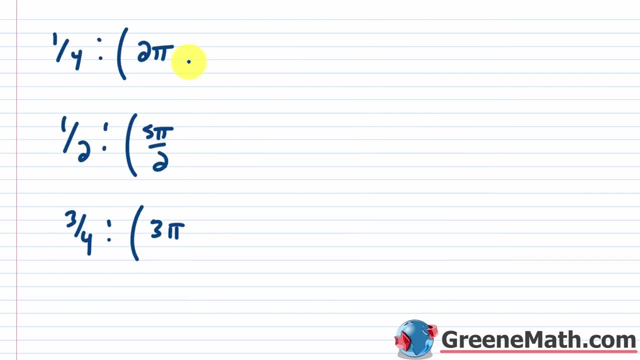 would be 3 pi, just doing 6 pi divided by 2.. Okay, we don't need this anymore. We have what we want. So, basically, all you need to do at this point is get your y coordinates And if we go back to the 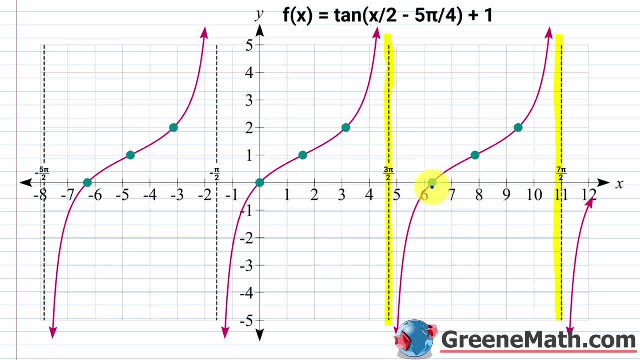 graph you can see that this right here is your first quarter and it's going to be at 0.. So you're on the x axis, then the midway or the halfway point you're going to be at positive one for the y coordinate And then for the three quarters of the way you're going to have a y coordinate of. 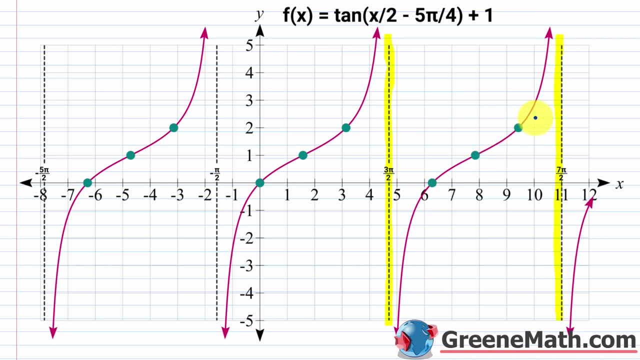 two. So it's going to be 0,, 1, and then 2.. Now, where's that coming from? Well, basically, you have to do a little bit of a vertical transformation. This right here is just a 1,, if you want to write. 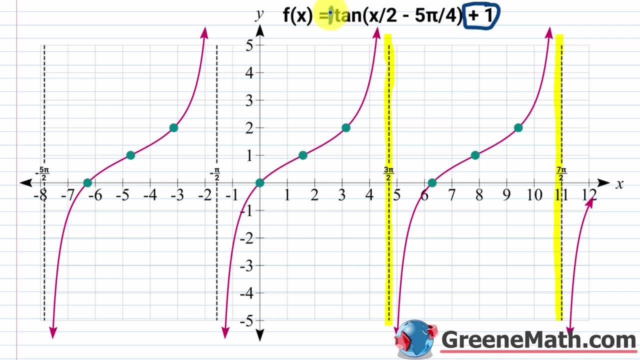 it. So, basically, all you have to do is take your normal y values, which you get negative 1,, 0, and 1, and just move them up by 1.. So, in other words, instead of negative 1, you get 0. Instead of 0,. 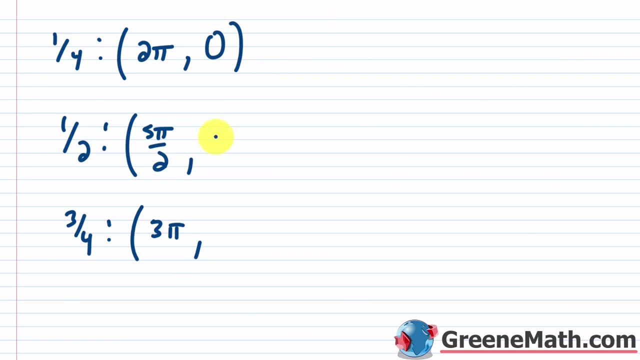 you get 1.. And instead of 1, you get 2.. This is going to be 0. This is going to be positive 1. And then this is going to be positive 2.. Again, that's coming from those basic points, from the. 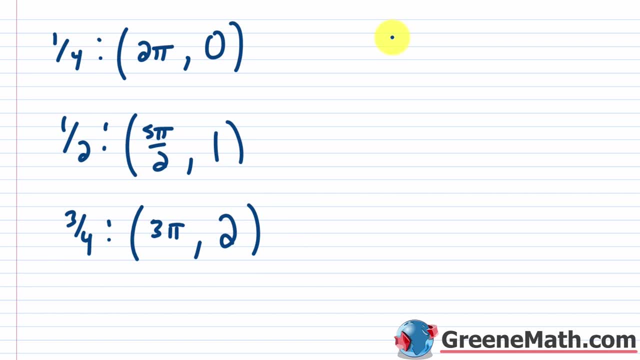 tangent graph. So negative pi over 4 comma. negative 1, your y coordinate of negative 1, you add 1, you get 2.. So you're going to have a negative 1, and then you get 2.. So you're going to have a negative. 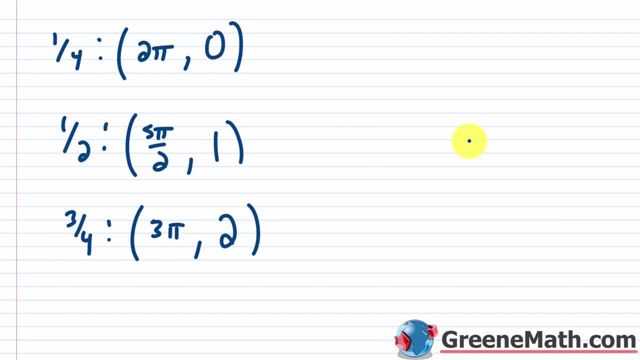 0. Then your halfway point is 0 comma 0. Your y coordinate of 0, you add 1,, you get to 1.. Then your pi over 4 comma 1, you take that y coordinate of 1,, you add 1,, you get to 2.. So those are your. 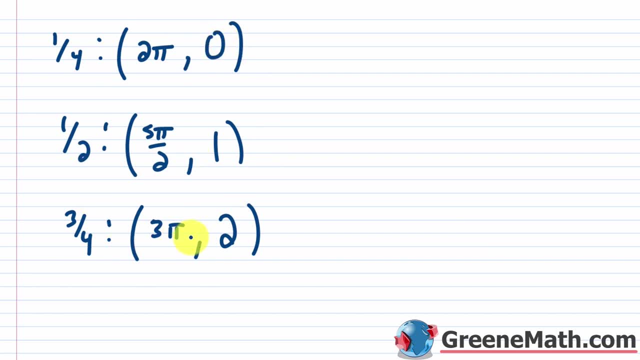 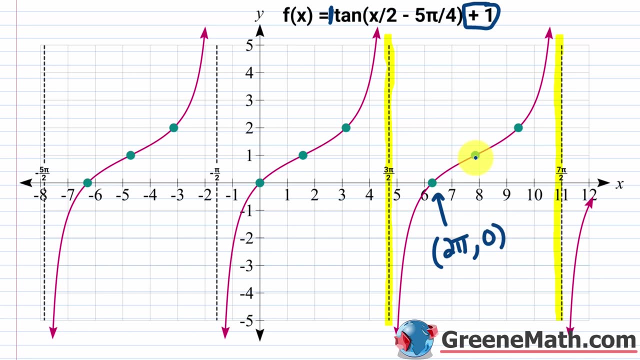 points for the quarter, half and three quarters. So you can have 2 pi comma 0. Let me label that. So this right here is 2 pi comma 0. Then this one right here is 5 pi over 2 comma 1.. So let me. 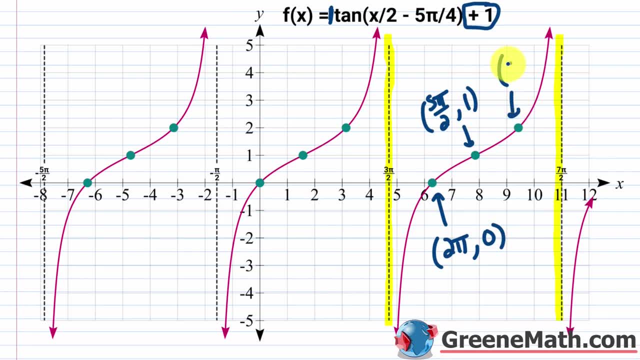 label that. So this one is 3 pi comma 2.. So this one is going to be 3 pi comma 2.. Now, in terms of continuing this graph to the left or to the right, remember that for these points you're always going. 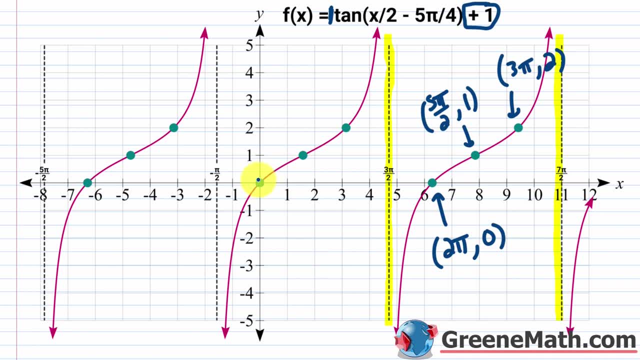 to have the same y value. So this one, the first quarter point- you're always going to have a y value of 0.. For the halfway, you're always going to have a y coordinate of 1.. For the three quarters way, you're always going to have a y coordinate of 2.. So that's not going to change. The only thing. 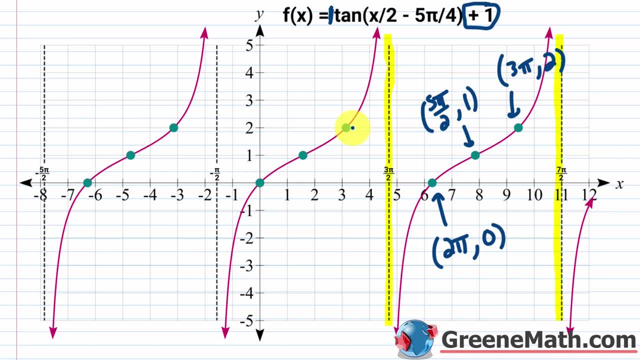 that's going to change is the x value, And the way you can do this is you can just constantly add if you're going to the right, or subtract if you're going to the left. So you're going to add or subtract if you're going to the left, quarter periods. That's all you really need to do to find. 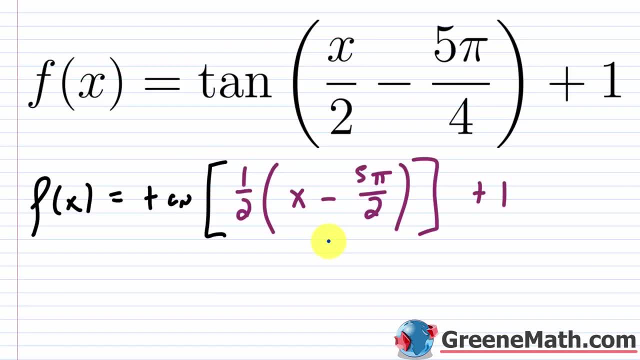 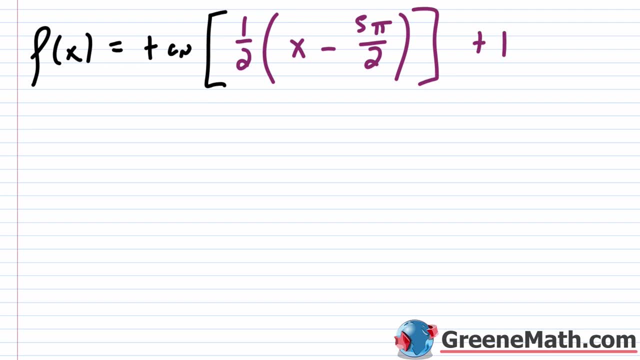 your additional points and your additional vertical asymptotes. Okay, so one more time I'll do this with transformations only. I know a lot of people want to see this because you don't get a chance to really practice this in the book because they don't cover it in most cases. So 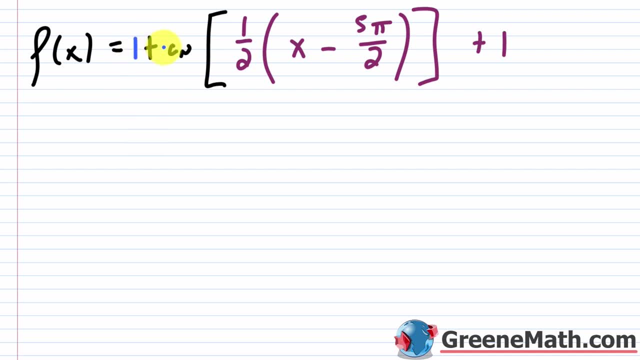 again, when I think about this, I can put a 1 right here. So really, in terms of a stretch or compression vertically, there's not right. So basically you have 1 times the tangent of whatever this is, and then plus 1.. 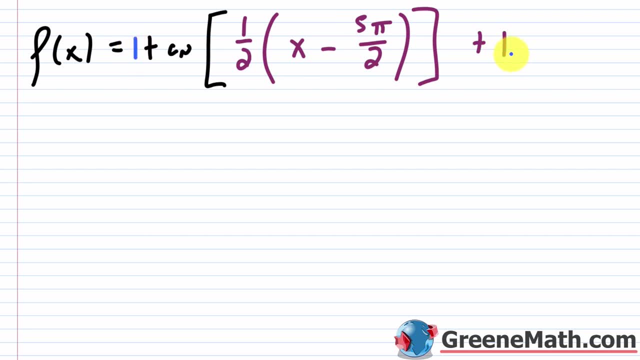 So there's no vertical stretch or compression. This is just a 1.. But you do have this plus 1 on the outside here, which is giving me a shift up by one unit. So in terms of the vertical transformations, I know that I'm just going up by 1.. Again, if you want to take these right here, 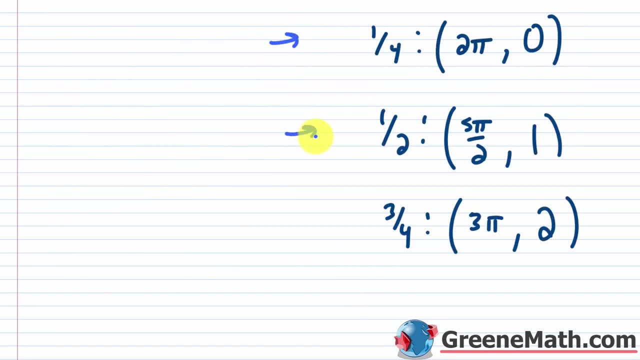 and let's slide this down and compare them to the original points: from y equals the tangent of x. let me do this like this: You have negative pi over 4, common negative 1, you have 0, 0, and then you have pi over 4, 1.. Well, again, all I'm doing is I'm just adding 1. 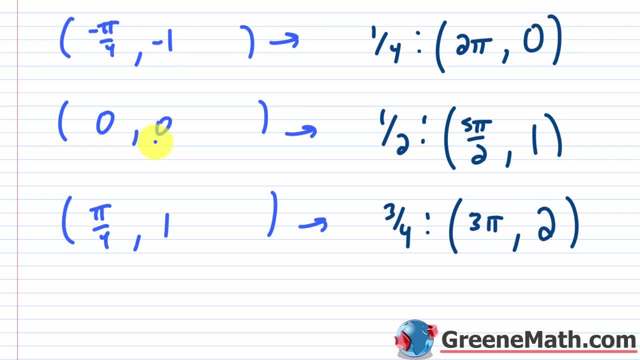 to each y value. So negative 1 goes to 0,, 0 goes to 1,, 1 goes to 2.. So we did that already, But basically that's all we're doing for the vertical transformations. Okay, let me put this: 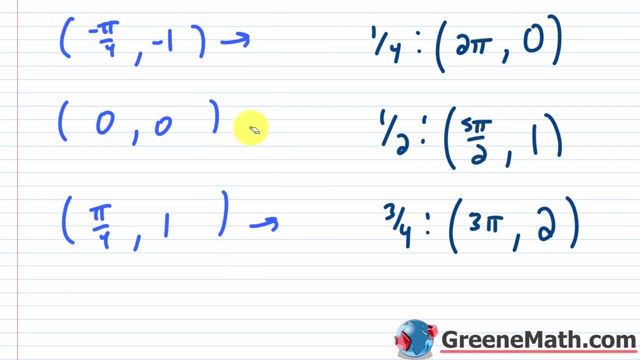 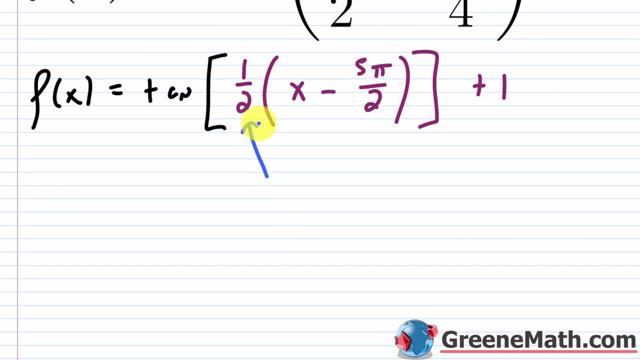 right here. And now let's talk about the horizontal. Again, this is the one that's a little bit more confusing And basically now we have the case where we have this one half here. So remember if it's between 0 and 1,. 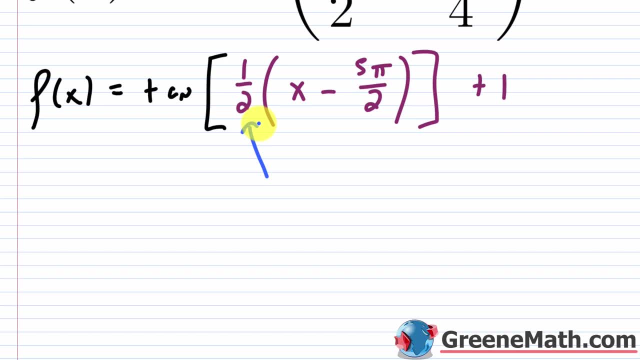 now you're getting a horizontal stretch Again. it's always the opposite of what you think. How do you undo multiplication by a half or dividing by 2? if you want to think about it that way, Well, you need to multiply by 2.. So the first step here, so step number 1, you're going to 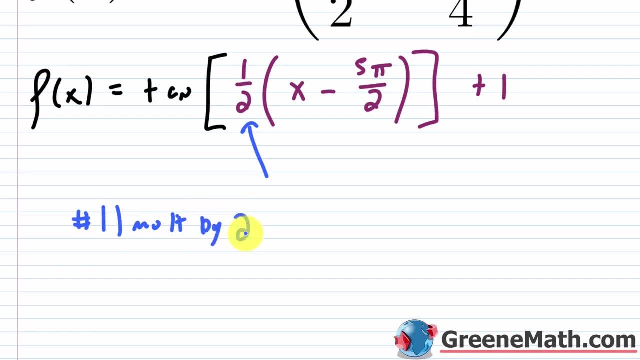 multiply by 2.. This is going to be horizontally stretched by a factor of 2.. And remember, this is going to be what you do first. Then this part right here: this is minus 5 pi over 2.. So this is going to be done second Again. 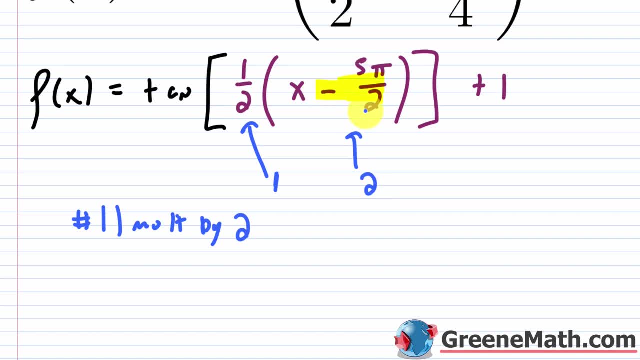 the reverse of what you think. So since this is minus 5 pi over 2, I've got to add 5 pi over 2.. So I want to shift to the right by 5 pi over 2.. Let me put for number 2, this is going to be add 5 pi. 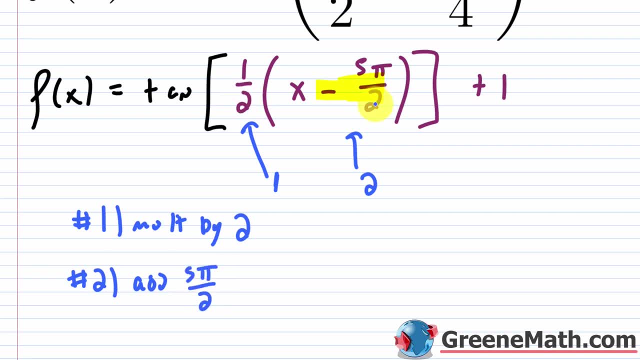 over 2.. So again, if you always remember that things on the inside are the reverse, So basically this is one half. So to undo that I need to multiply by 2. This on the inside is minus 5 pi over 2. To undo that I need to add 5 pi over 2.. And then you even go in the reverse order, So you: 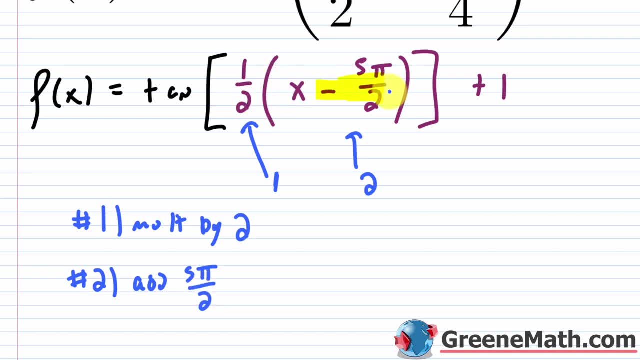 reverse the order of operations. Normally you do what's inside a parentheses first and then you would multiply second. you reverse that order, So you would do this one first. you do the multiplication first and then you do this part right here, what's inside the parentheses second. So you have to 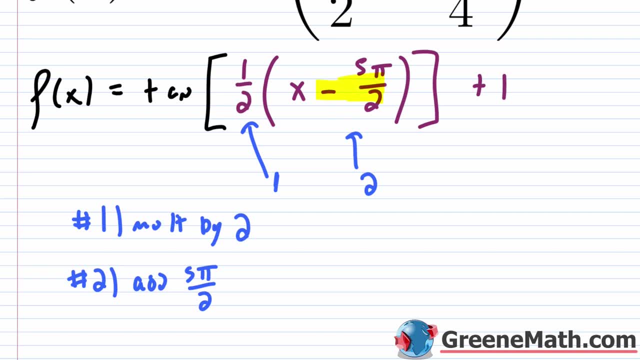 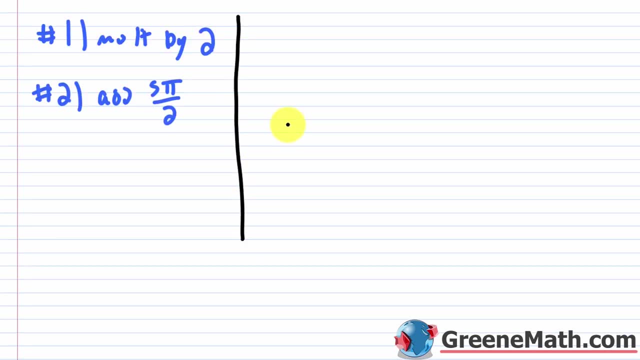 keep everything straight. with the horizontal transformations I know it gets super confusing. So if this is not something that's straight in your mind, I would just go with the other procedure. You could start off with the vertical asymptotes, So just start with your. x equals negative pi over. 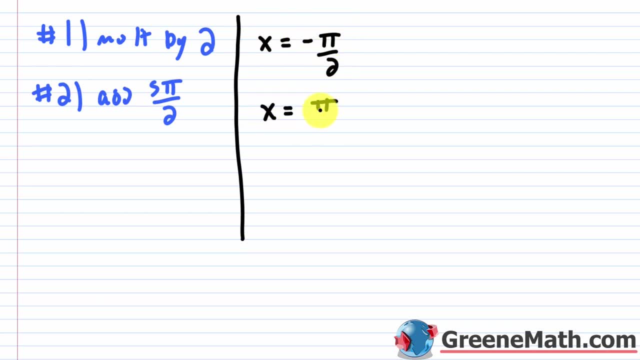 2. And x equals. you could do pi over 2. Like this. So these are your vertical asymptotes when you think about the standard y equals tangent of x that you start with. So basically, I'm going to multiply by 2 first, So let's go. 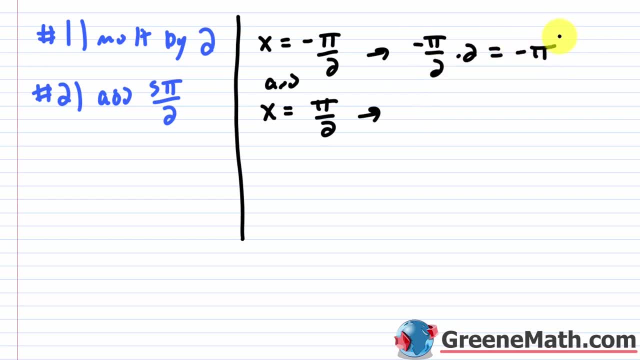 negative pi over 2 times 2. That's going to give me negative pi. Then, once I've done that, I want to add 5 pi over 2.. So let me start now with negative pi like this And I'm going to add 5 pi. 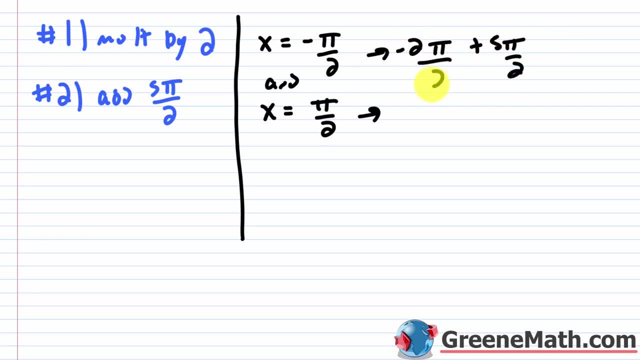 over 2.. Well, let's write this as negative: 2 pi over 2.. And what is that going to give me? Negative 2 pi plus 5 pi, that's 3 pi, And then, over the constant, I'm going to add 5 pi over 2.. So that's. 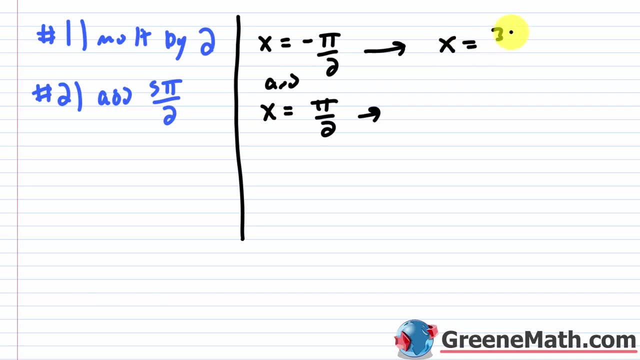 a common denominator of 2.. So this would go to: x is equal to 3 pi over 2.. Then for this one again, you're going to multiply by 2, first Pi over 2 times 2.. Let me show this so nobody's lost That. 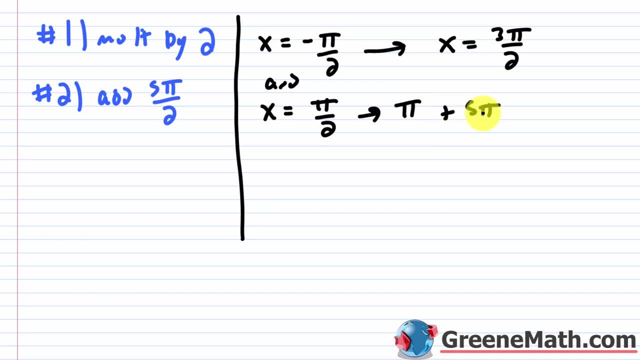 would give you pi, And then you're going to add 5 pi over 2.. So write this as 2 pi over 2.. You add that together You're going to get 7 pi over 2.. So this right here is going to become: x is equal to. 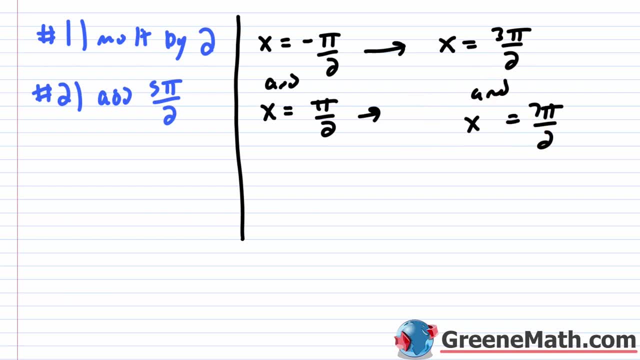 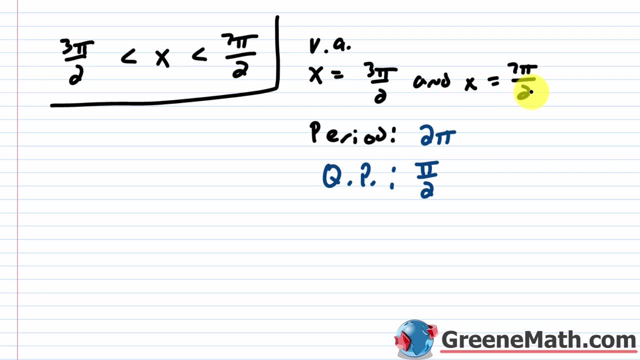 7 pi over 2.. Let me put and there And again. if you go back and check, we found from the other side that x is equal to 3 pi over 2 and x is equal to 7 pi over 2.. Those are your vertical. 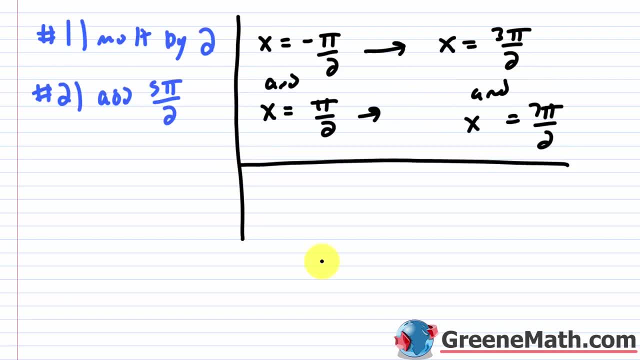 asymptotes. Now for the other x values again from that first quarter point. from y equals tangent of x, you have an x value of negative pi over 4.. So you take negative pi over 4. You multiply by 2 first. This would cancel. That gives you 2 down there. So this would be equal to: 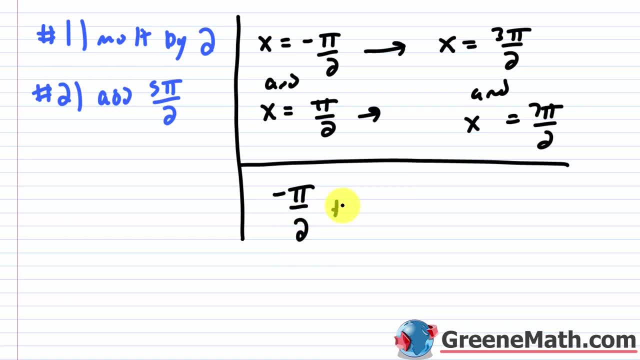 negative pi over 2.. And then from there you're going to add 5 pi over 2.. So this would give me 4 pi over 2.. Again, if you look here for the first quarter point, you have an x coordinate of 2 pi Again. 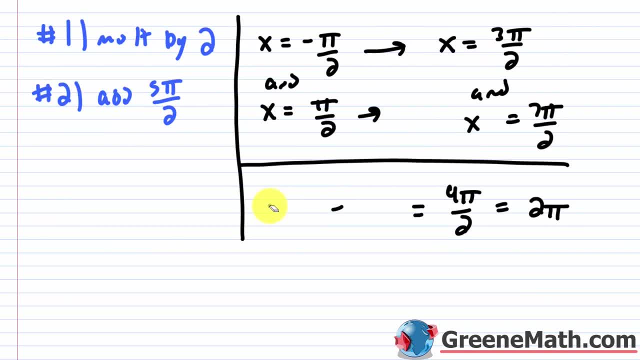 we already figured out that the y coordinate was 0.. Now for the next one, you have an x coordinate of 0. So you multiply that by 2. I don't even need to show that That's still 0. And then you add 5 pi over 2.. That's going to give you 5 pi over 2.. So see our x coordinate. 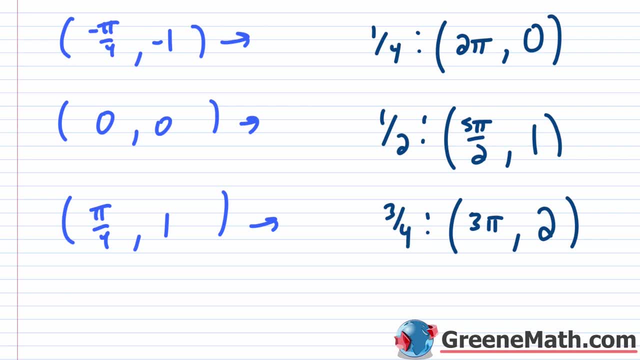 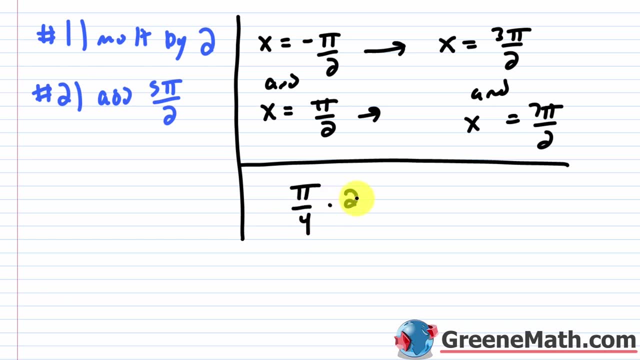 here is 5 pi over 2 for the midway point. So we just need the last one. So you have pi over 4 for that, 3 quarters of the waypoint for the x value, And again I'm just going to multiply by 2.. 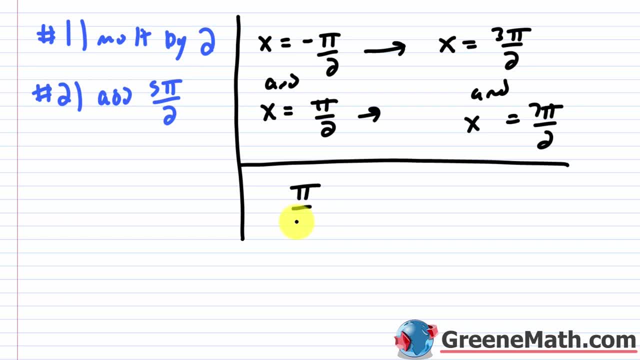 So this would cancel. It's going to be 2 down there. So now I have pi over 2.. And then, once I've done that, I'm going to add 5 pi over 2. And this becomes 6 pi over 2, which is 3 pi. 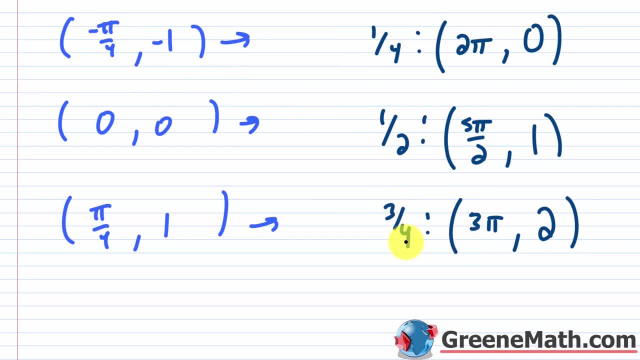 So again, you come over here and confirm with what we already did For the 3 quarters point: you're going to get 3 pi for the x value. So that's an alternative approach. if you just want to use graphing transformations, As I told you in the last example, I know a lot of students. 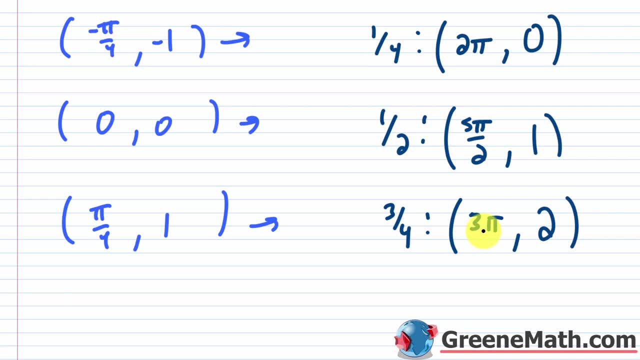 struggle with it, particularly with the horizontal transformations, because everything is the reverse. So I'm going to add 5 pi over 2.. And then, once I've done that, I'm going to add 5 pi over 2.. And then, once I've done that, I'm going to add 5 pi over 2.. So again, you can. 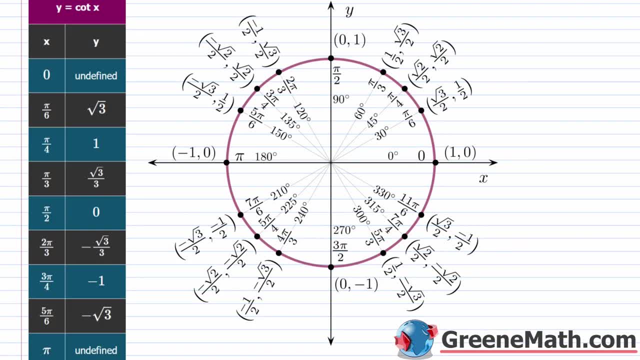 say counterintuitive to what you think. All right, let's talk about the cotangent function now. So most of you know that the cotangent of x is equal to the cosine of x over the sine of x. So again, just like we saw with our tangent function, the period is pi. You could take 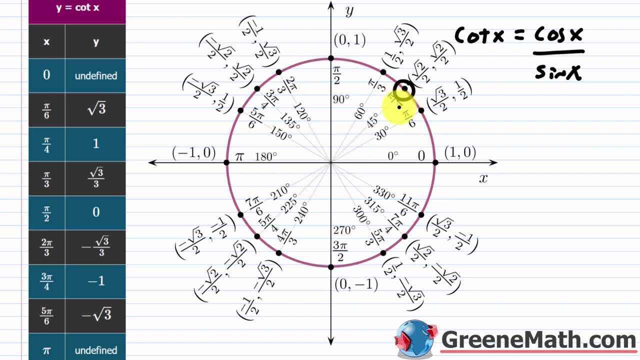 this point right here, which is pi over 4, and the cotangent value would be 1.. You're dividing square root of 2 over 2 by square root of 2 over 2.. This is your cosine value. this is your sine. 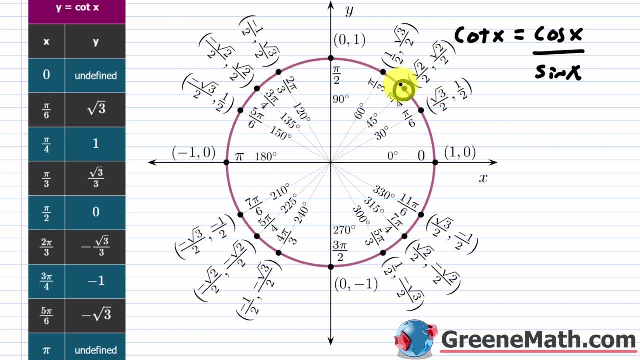 value. the same non-zero number divided by itself would be 1.. If you swing around by pi, so you add pi and you go to this 5 pi over 4, which is right. here again you're dividing the same non-zero. 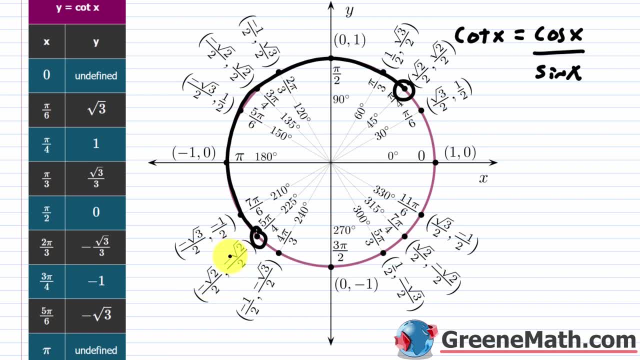 number by itself. Here you have a negative square root of 2 over 2, and here you have a negative square root of 2 over 2,, so you're still going to get 1.. And the same thing would be true if you. 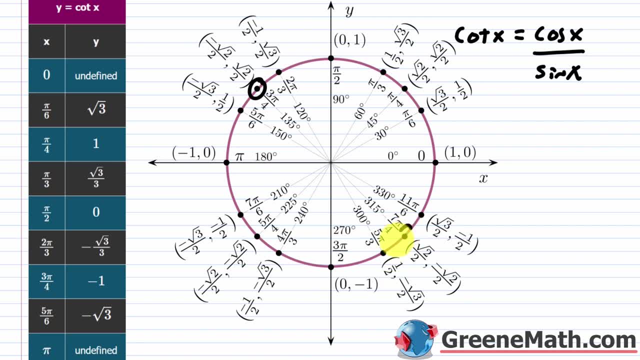 looked at, let's say, 3 pi over 4, and then you looked at 7 pi over 4.. Well, here the cotangent value is negative 1, because you're dividing opposites. So if you swing around, you're going. 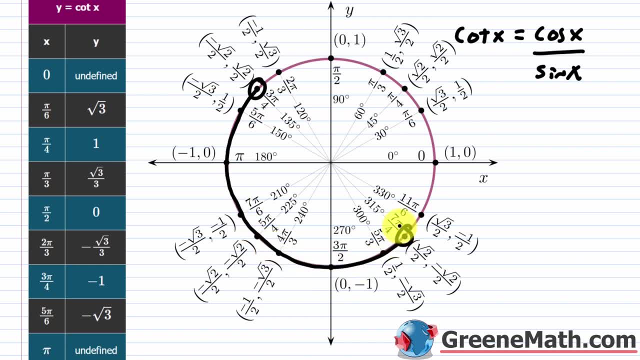 to see, the cotangent value is negative 1 there as well, at 7 pi over 4.. So the period here is going to be pi again, just like with tangent, When we think about the fact that cosine of x is now in. 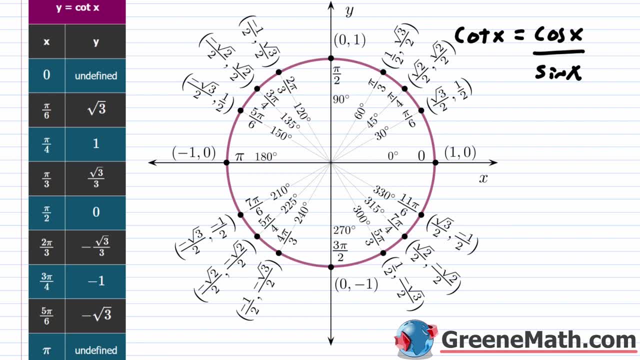 the numerator. well, anywhere where the cosine value is 0, so again we know that's at pi over 2, 3 pi over 2,, 5 pi over 2, or you could go negative pi over 2,, negative 3 pi over 2,. 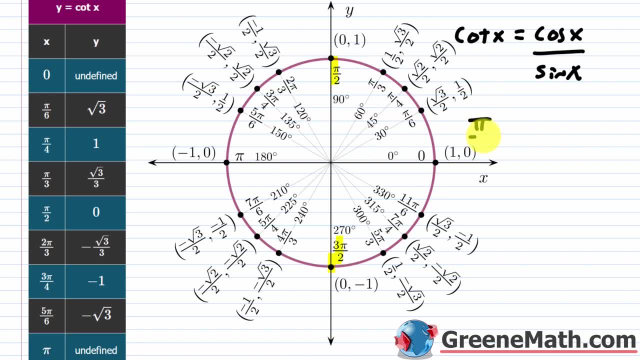 basically odd multiples of pi over 2, or you can say pi over 2 plus pi n, where n is any integer. That's going to be where the x-intercepts are now. So basically, that's where this is going to be 0, and this will not be 0.. So 0 divided by something that's not 0 will give you 0.. 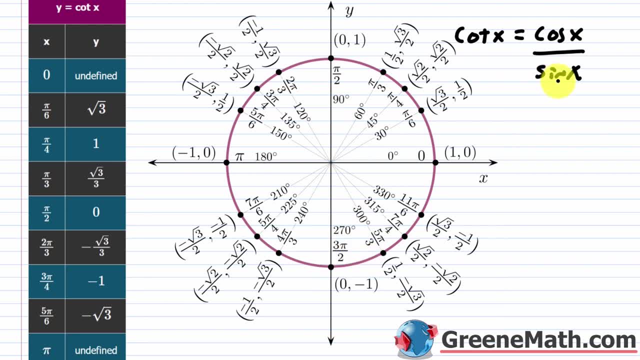 Then, in terms of where it's going to be undefined, well, that's going to be where the sine values are 0, because again, that gives you division by 0. So that's going to be right here at 0, then at pi, then at 2 pi, 3 pi, or you could have negative pi, negative 2 pi. 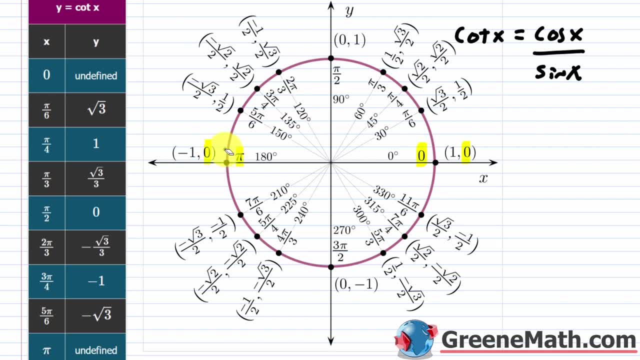 So basically you would say pi n where n is any integer? Now I have a few basic points here. so, just like we saw before, So we have at 0, this guy's undefined again because your sine value is 0. Then at pi over 6, you're going to get. 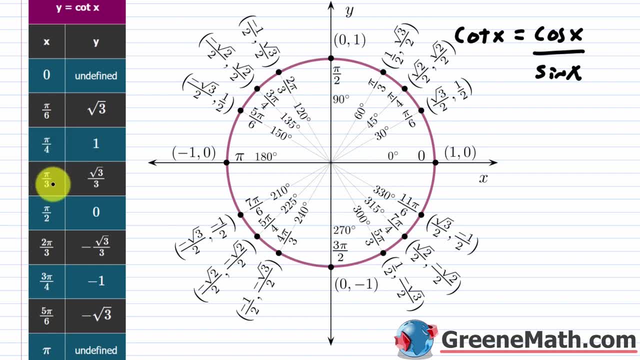 square root of 3.. At pi over 4,, you're going to get 1.. At pi over 3,, you're going to get square root of 3 over 3.. At pi over 2, you're going to get 0.. At 2 pi over 3,, you're going to get negative. 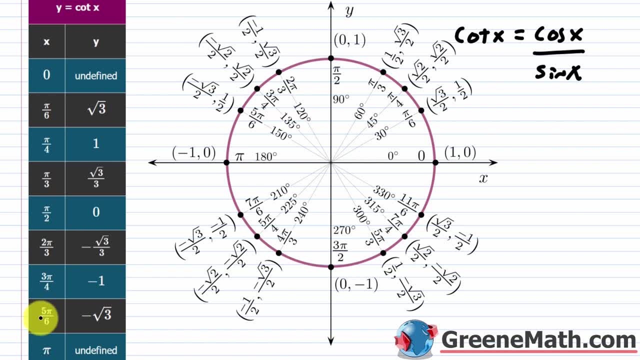 square root of 3 over 3.. At 3- pi over 4, you're going to get negative 1.. At 5- pi over 6, you're going to get negative square root of 3.. And then at pi, you're going to get undefined. So we're. 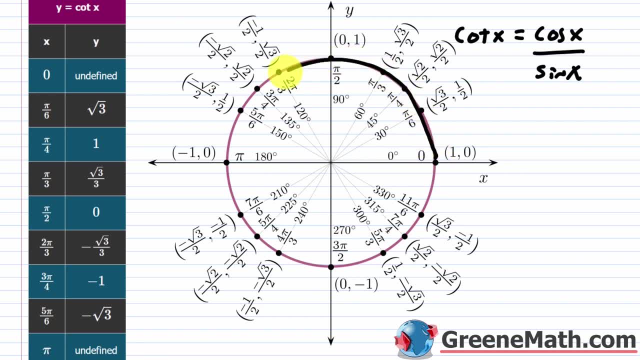 going to graph this over the interval from 0 to pi, with both of those being excluded, because again, at 0, it's undefined and at pi it's undefined, So again we're going to get vertical asymptotes at those values. All right, let's take a look at a basic sketch of. y equals the cotangent. 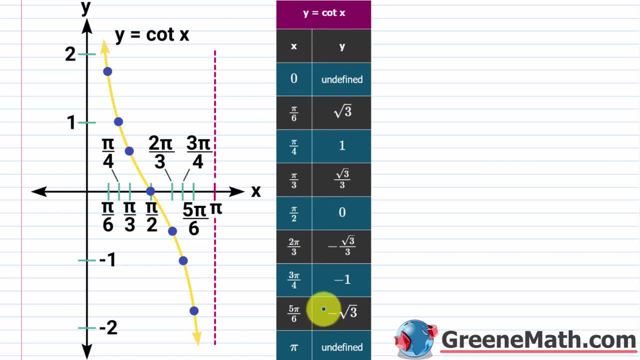 of x, just using these points right here. Again, when you first do the graph of this, you're just going to work from 0 to pi, with both being excluded, So you can see that at an x value of 0,. 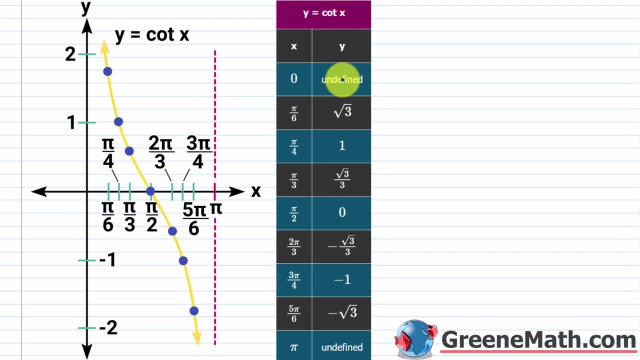 the y value is undefined because if you have cotangent of 0,, you have the cosine of 0,, which is 1,, over the sine of 0,, which is 0, and 1 divided by 0 is undefined. 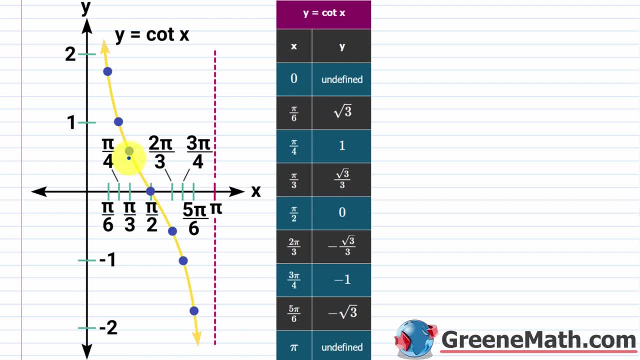 So that's why you get undefined Again as this guy approaches an x value of 0,. so, coming from the right, as we do this, this guy is going to increase without bound, So it's going to approach positive infinity. Then, similarly for an x value of pi, again the cosine of pi is negative: 1,. 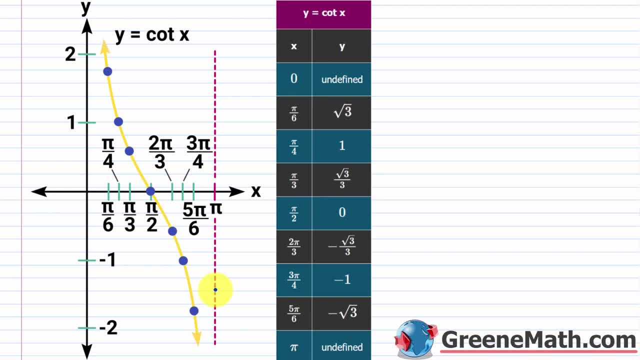 and the sine of pi is 0. So if I say I want the cotangent of pi, you're setting up the fraction negative 1 over 0, that's going to be undefined. So as your x value approaches pi coming from the 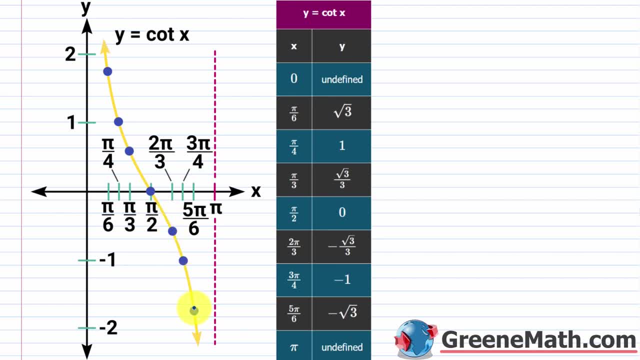 left. so, coming from the left, going this way, you're going to get undefined. So you're going to: this is going to decrease without bound, we're going to approach negative infinity. Now, in terms of this stuff in between, you have pi over 6, comma, square root of 3.. So here's your pi over 6 for the 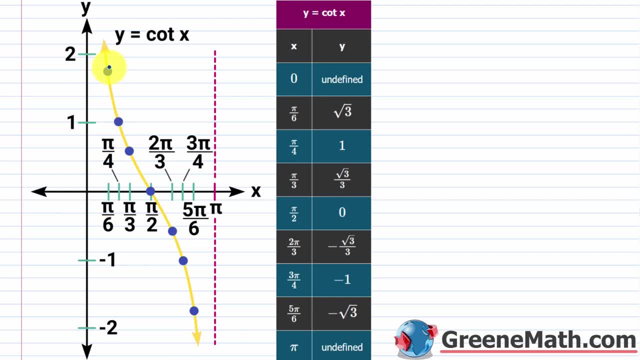 x value, this would be square root of 3 for the y value. So this point right here is: pi over 6 comma square root of 3.. Then you have your pi over 4 comma 1.. So this is one that you want to. 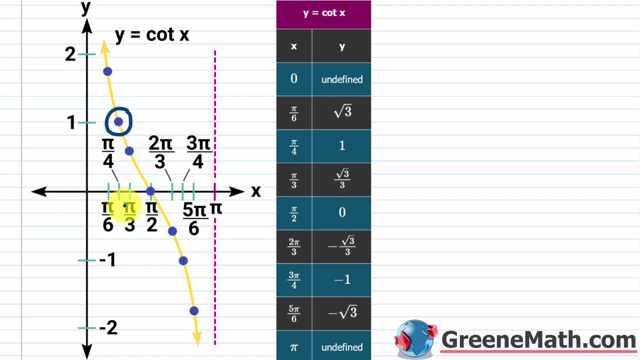 memorize: that's going to be your first quarter point. we're going to use that. Then you have your pi over 3 comma, square root of 3 over 3.. So it's going to be this guy right there Then you. 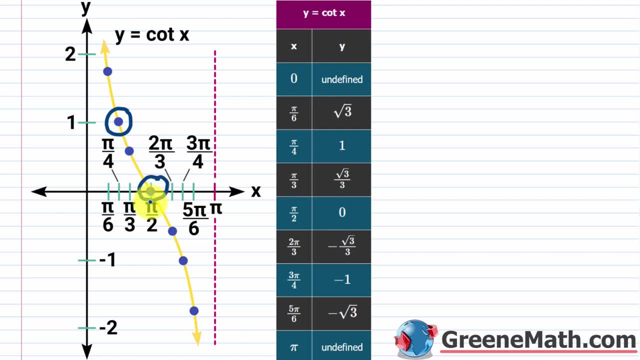 have your pi over 2 comma 0.. So this is your halfway point, So you need to memorize that one. Then you have your 2 pi over 3 comma, negative square root of 3 over 3.. So that's this point. 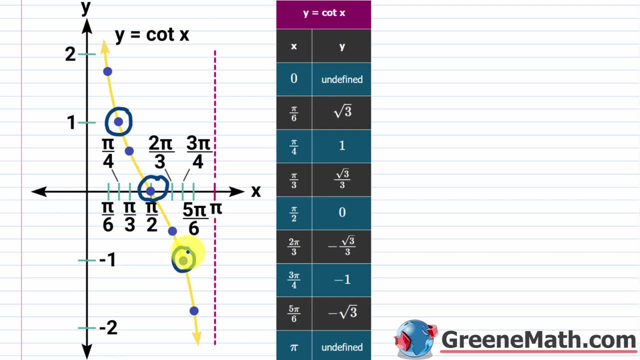 right here. Then you have your 3 pi over 4 comma negative 1.. So that's going to be this point, right there. That's going to be three quarters of the way through, So that's one that you need to memorize. And then, lastly, you have this 5 pi over 6 comma negative square root of 3.. So that guy. 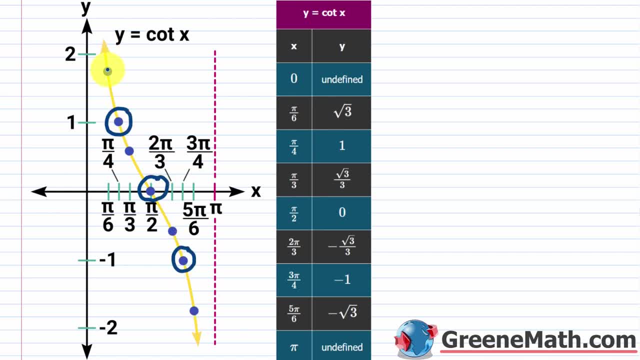 right there. So that's your basic points. Usually you just put this point, this point and this point. you make a vertical asymptote here. you don't need to make one here. you can if you want, But typically you leave that off because this is the y axis. so you don't. 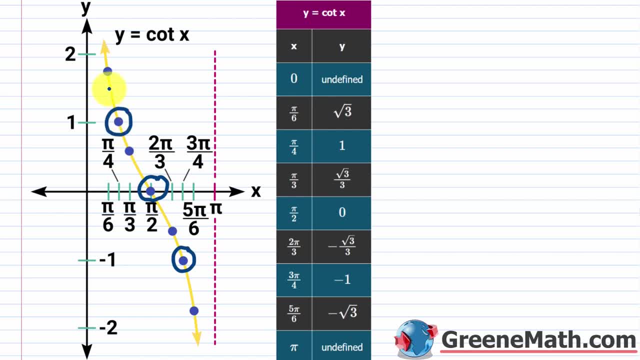 draw anything And basically you just draw this to where it approaches the y axis and doesn't touch it. And this guy is going to approach this vertical asymptote, which is x equals pi, but not touch it. So that's all you really need to do. So just like with the graph for y equals. 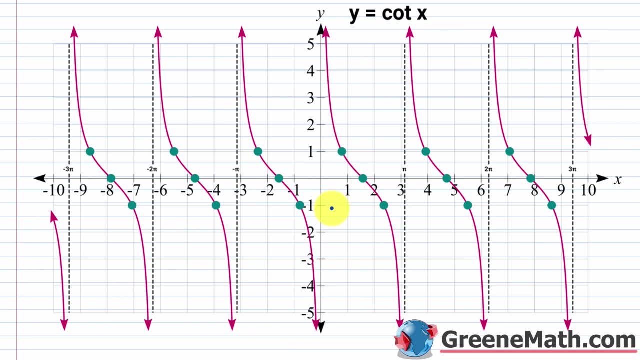 the tangent of x. when you expand this to the right or to the left, all you're doing is just copying what you previously did. In other words, we graph this right here. So from 0 to pi, with both being excluded, but basically the same thing is going to happen: from pi to 2 pi, 2 pi to 3 pi. 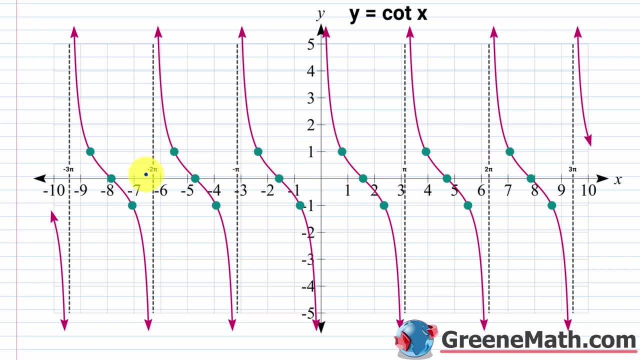 or if you went this way, you can say from negative pi to 0,, you could say from negative 2 pi to negative pi, so on and so forth. So you're going to have a vertical asymptote. you're going to have 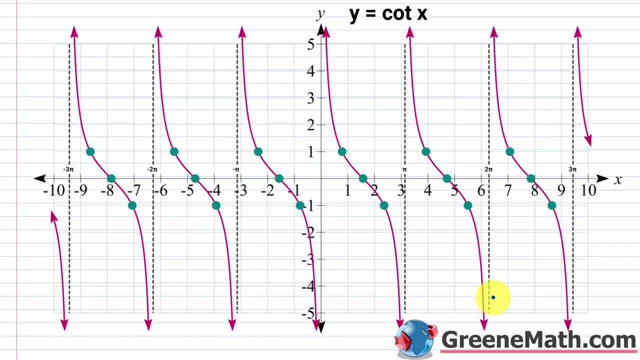 three points: vertical asymptote. So it's just that pattern, over and over and over again, And these three points again. the benefit to these guys right here is that basically, all you need to know is what is the vertical asymptote here And what is the vertical asymptote here? So I'll 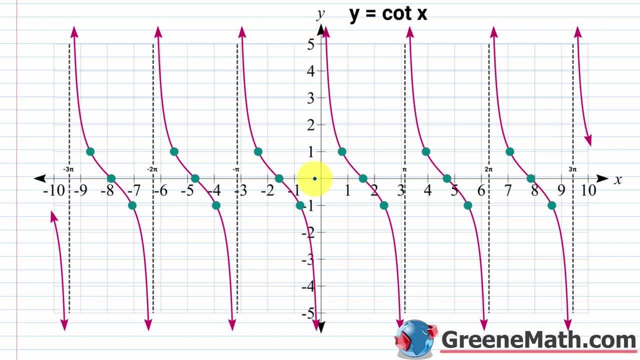 show you how to get that in a moment, Once you have this one right here on the left. in this case it would be zero. you just add a quarter period. Well, a quarter of the normal period for cotangent is pi. So a quarter of that is pi over 4.. So I know the x value right here is pi. 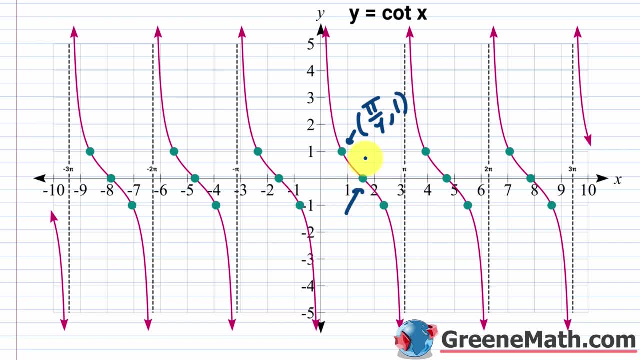 over 4.. And of course the y value is 1, we can see that. Then this one: right here again, you just add a quarter period. So pi over 4 plus pi over 4, that's 2 pi over 4, or pi over 2, and the y value. 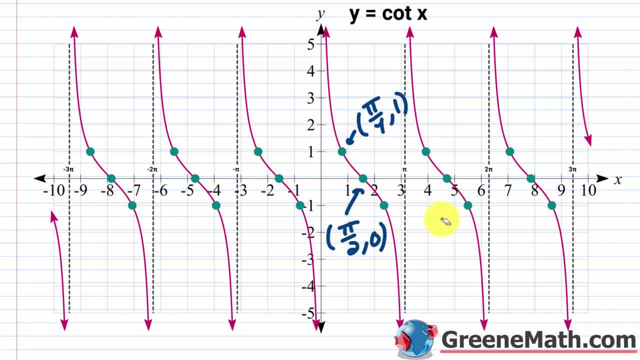 is 0.. Then for this one again, I'm just adding a quarter period. let me make that arrow better. So if you have, let's go 2 pi over 4, so we have a common denominator plus pi over 4,. 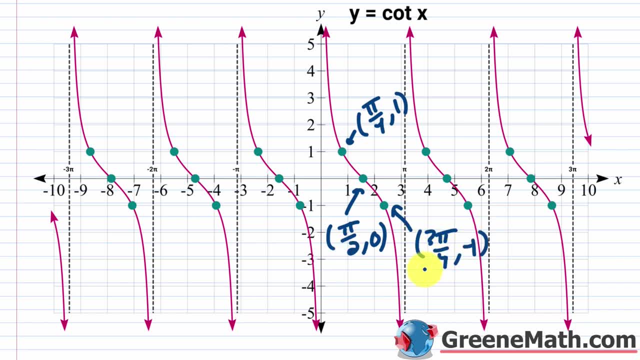 that's going to be 3 pi over 4, comma negative 1 for the y value. So the y value are things that you want to memorize because typically you're going to do this with graphing transformations. So if you know those y values it's going to save you a lot of time you can. 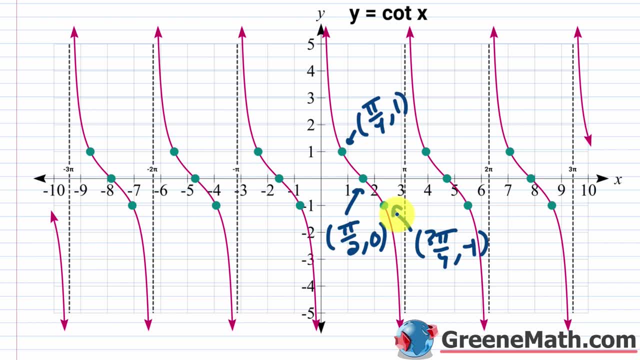 always plug in if you want to, but I find that to be a very tedious process. For the x values again, all you're gonna have to do is find the vertical asymptotes, figure out the period and the quarter period and then just go through the process of adding quarter periods to get to the 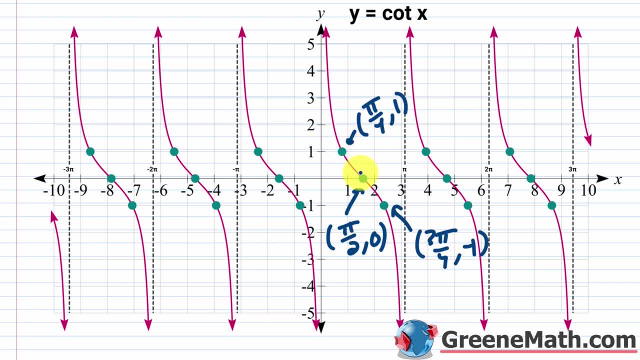 next x value. So start here, add a quarter period. I get to this x value. add a quarter period. add a quarter period. add an asymptote. add a quarter period. add a quarter period. add a quarter period. add an asymptote. So when 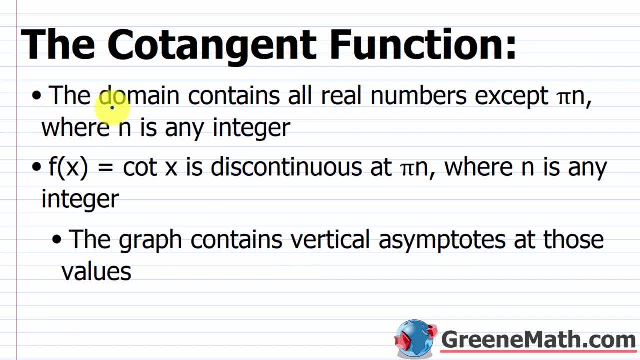 and so forth. All right, let's talk a little bit about the cotangent function in general. So the domain contains all real numbers except for pi n, where n is an integer, So 0, pi, 2 pi, 3 pi, or even negative pi, negative 2 pi, that's where the sine value is zero. And again division. 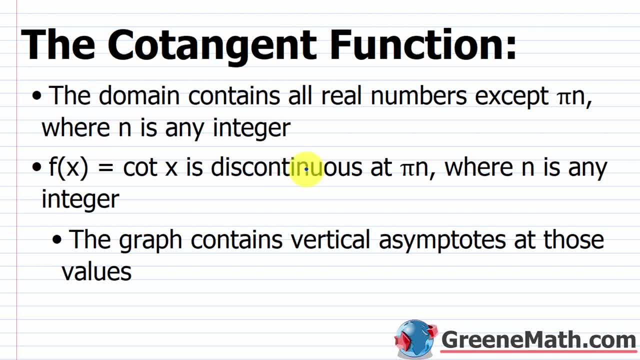 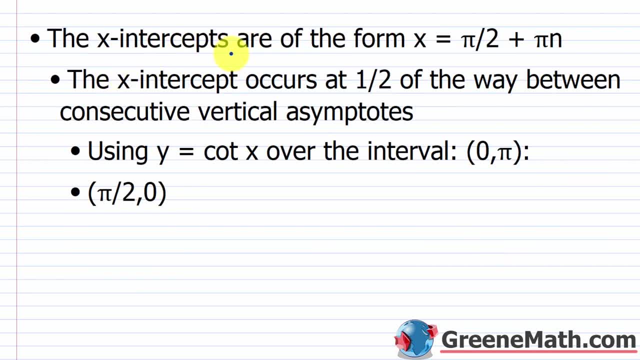 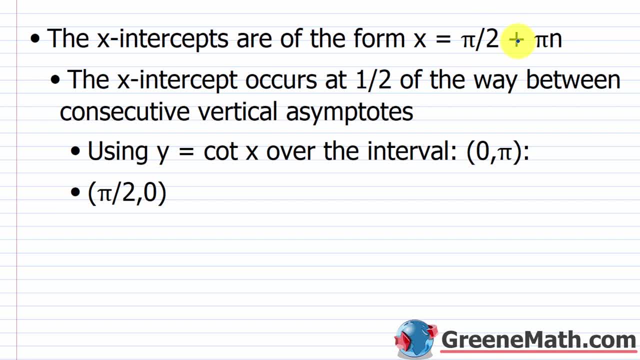 are of the form f of x and the denominator is not zero. So these are of the form f of x and the denominator is not zero. Remember that cosine of pi over two is zero, And then plus pi n, where n is any integer. The x intercept occurs at half of the way between consecutive vertical. 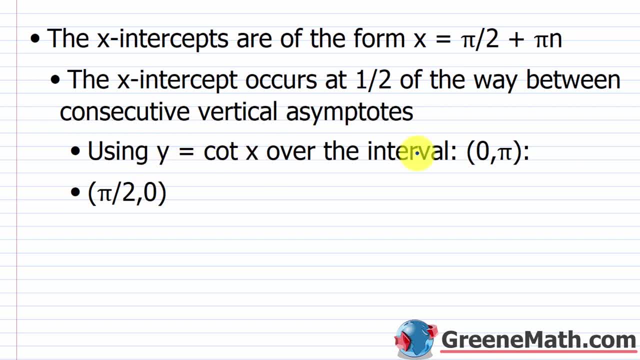 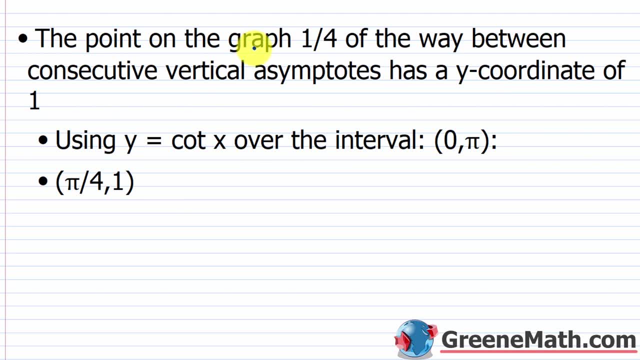 asymptotes. So if we use that basic, y equals cotangent of x over the interval from zero to pi. both being excluded, this is going to happen at pi over two comma zero. So you want to memorize that point? then the point on the graph one: fourth of the way between consecutive vertical asymptotes. 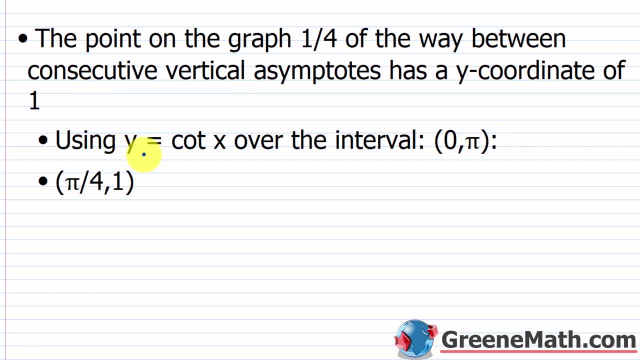 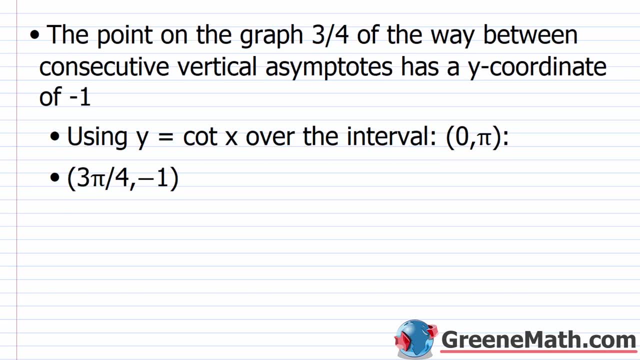 has a y coordinate of one. So we saw that already. So if you're using y equals cotangent of x over the interval from zero to pi, with that Y that's going to be equal to y equals cotangent of x over, with both being excluded. well, you're going to have pi over 4 comma 1.. Lastly, the point on the 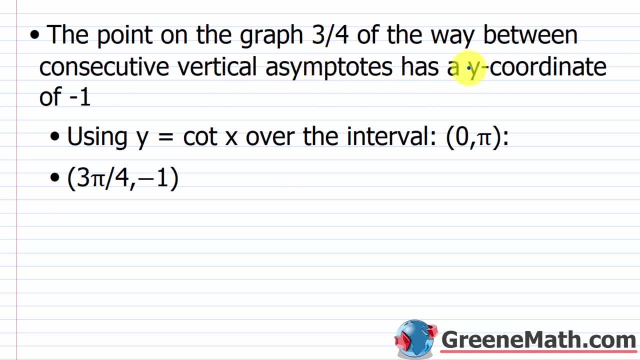 graph, three quarters of the way between consecutive vertical asymptotes has a y-coordinate of a negative 1.. Again, using y equals cotangent of x over the interval from 0 to pi. with both being excluded, you saw that we had 3 pi over 4 comma negative 1.. So again, the period is pi. There are 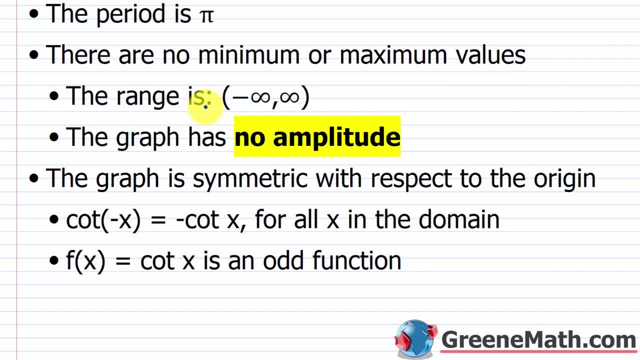 no minimum or maximum values. The range is from negative infinity to positive infinity and the graph has no amplitude. So the graph is symmetric with respect to the origin. So if you did cotangent of negative x, it's equal to the negative of cotangent of x for all x in the domain. So f of 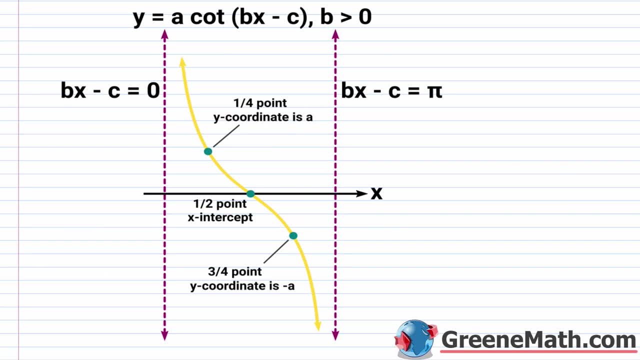 x equals the cotangent of x is an odd function, So, just like we saw with tangent, I gave you a little model you can use. It's not going to fit perfectly with every scenario, but we can just adjust it. So we have: y equals a cotangent of bx minus c, where b is greater than 0. Again, if b, 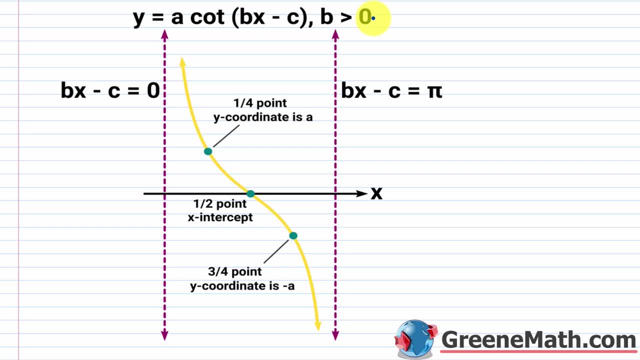 is negative, which you'll see in the future, you can rewrite it using identities. If you need the period, you can just use absolute value bars. It's really not that big of a deal. It won't cause that much concern. So what we would do is say that. 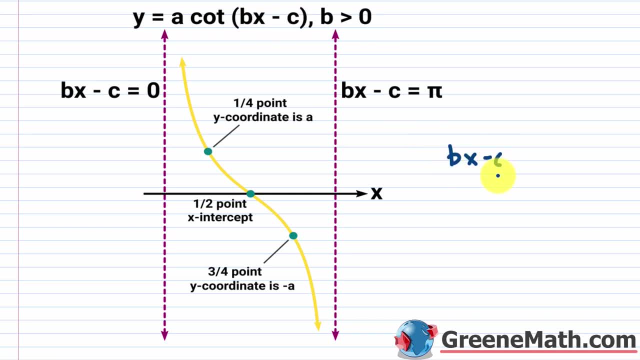 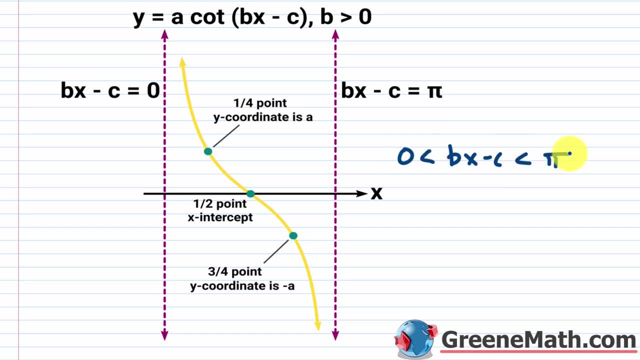 you're going to graph it by saying it's greater than 0 and less than pi, And that's coming from the fact that, if you have, y equals the cotangent of x. where we said that we're going to go, x is greater than 0 and less than pi. So, again, all you're doing is you're taking this argument right. 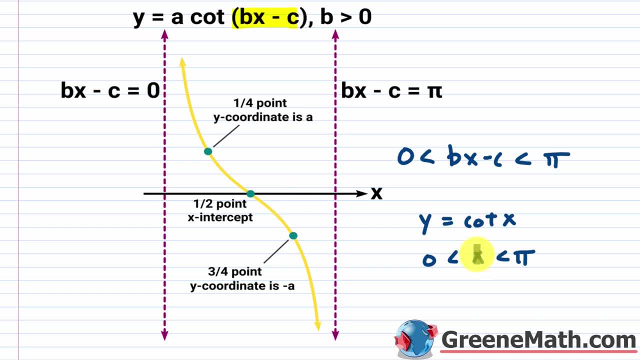 here, which is the bx minus c, and you're just putting it in that place right there, and you're going to solve for x. That's all you have to do. So, basically, once you've done that, you're going to find these two vertical asymptotes. So you could do that by doing this. You could do that by: 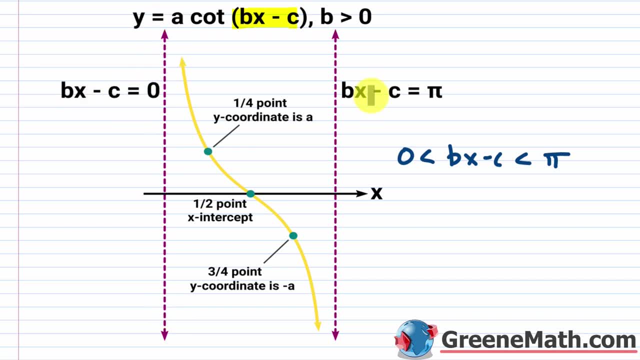 as an equation, bx minus c is equal to 0. So that's for this one. And then bx minus c is equal to pi for this one. And then, once you have that, just like with the tangent function, you can figure out what the period is. So it's just going to be pi over b. Let me write that out. So the 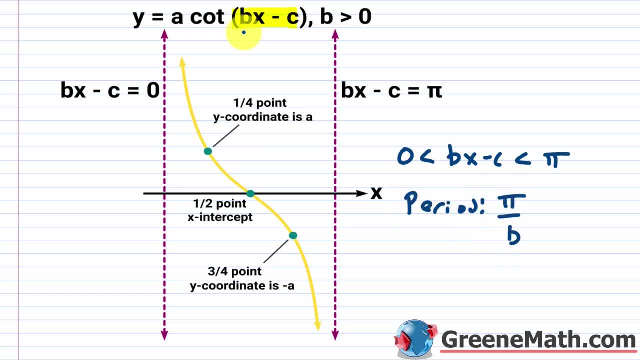 period is just pi over b. So whatever that is that coefficient of x if you end up factoring that out. so if you have something like y equals a cotangent of. let's say, we pull the b out because we want to use graphing transformations. Let me move this up so it fits. So then inside you would: 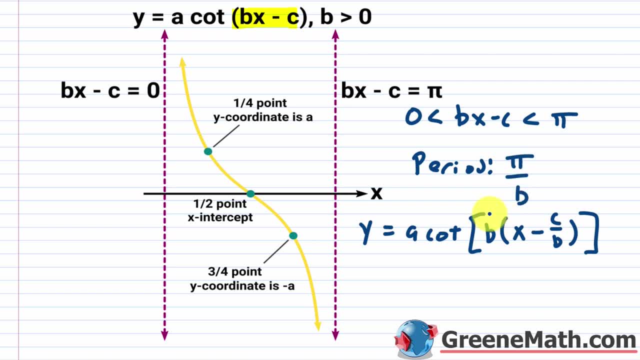 have x minus c over b, like that, Well, the period is still pi over b. So in this form it's the coefficient of x. In this form it's outside of the parentheses. So just keep that in mind Now. 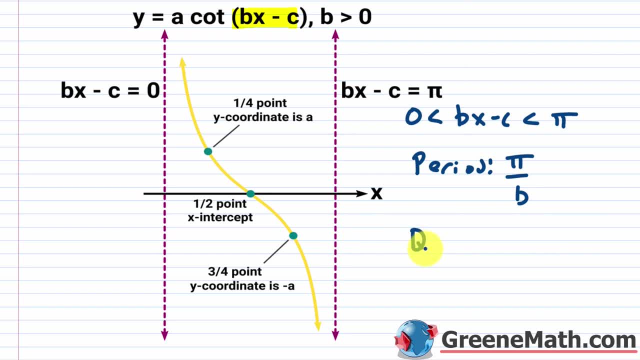 once you have that period you can just figure out the quarter period. So the quarter period again, that is just pi over 4b. So just take this and multiply it by a fourth. And once you have that you take the x value here, you add a quarter period, you're going to get your x value here. 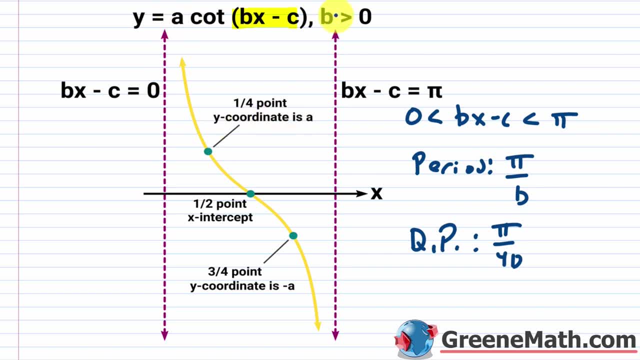 So the y coordinate would just be given by a in this form. But again, if you have a shift you have to consider that as well. You do this multiplication here first by your typical y coordinate, for y equals cotangent of x, which in that case is going to be positive one, And then 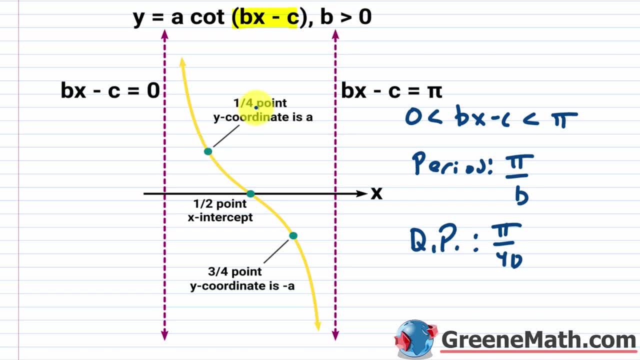 once you've done that, you need to apply your shift either up or down. This one fourth point: the y coordinate is a, because again, one times a would be a. Then, at the halfway point, the x intercept. well, again, I could just add a quarter period to get the x value there, And then for the 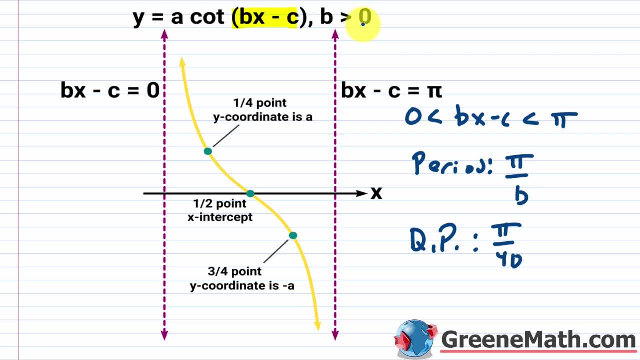 y value. in this form it's just going to be zero. But again, if you have a shift up or down you have to consider that. Then you add another quarter period to get the x value And then you're going to have your three fourths point And the y 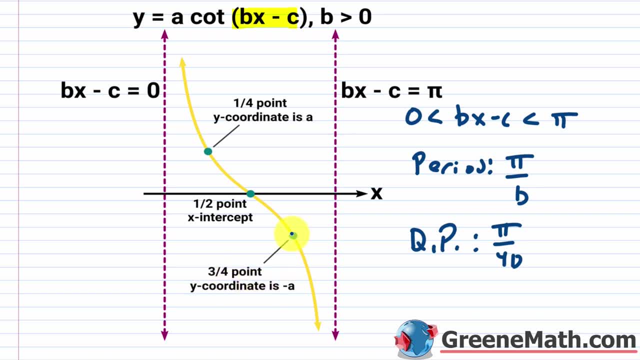 coordinate is now negative a, Because normally if you have y equals cotangent of x, three quarters of the way through you have that three pi over four comma negative one. So if you take that negative one, you multiply by a, you get negative a. That's where that's coming from, So just keep. 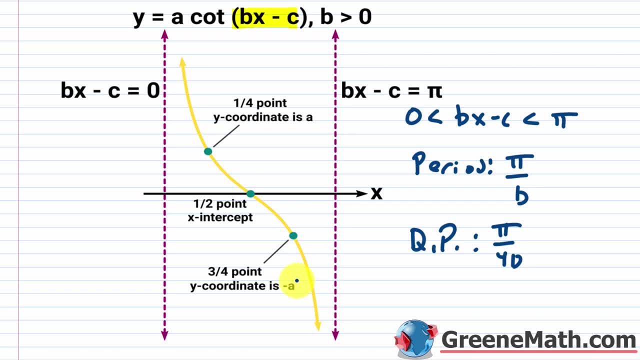 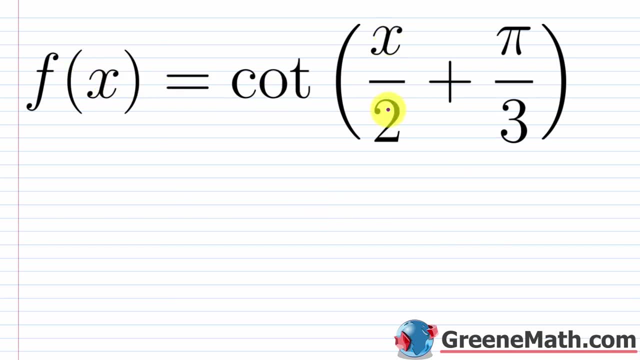 this in mind as a general model And, with that being said, let's just go ahead and look at an example. All right, let's take a look at an example now with cotangent. So we have: f of x equals the cotangent of x over two, plus pi over three. 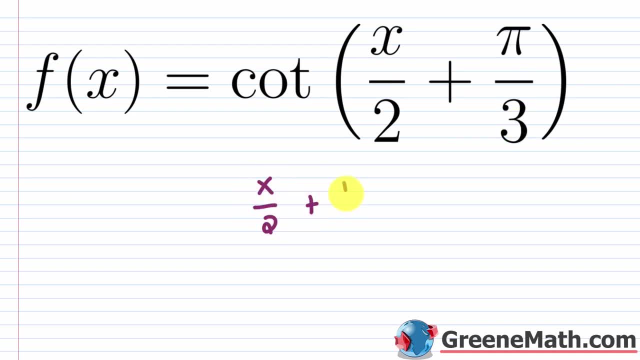 To start things off, I'm just going to go x over two plus pi over three. So that's going to be the argument for the cotangent function there. this guy And basically you're going to say that this is greater than zero and less than pi. So I'm going to get rid of these fractions here. You. 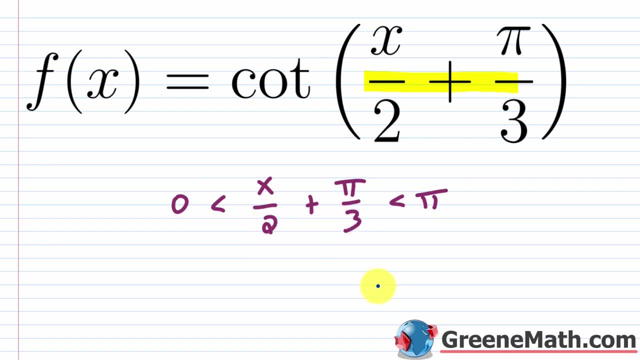 have a denominator of two and a denominator of three. So what I would do is just multiply both sides by the LCD, which would be six. So zero times six would still be zero. Let me just show it for right now. Multiply this by six. multiply this by six. Let me slide this over here. 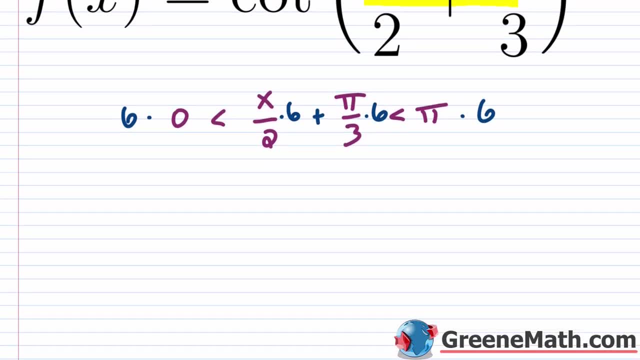 And then multiply this by six. Let me drop down a little bit. So, as I just said, zero times six is still zero. This is less than six divided by two would be three, And three times x is three x, And then plus six divided by three is two. Two times pi is two pi, And then this is less than. 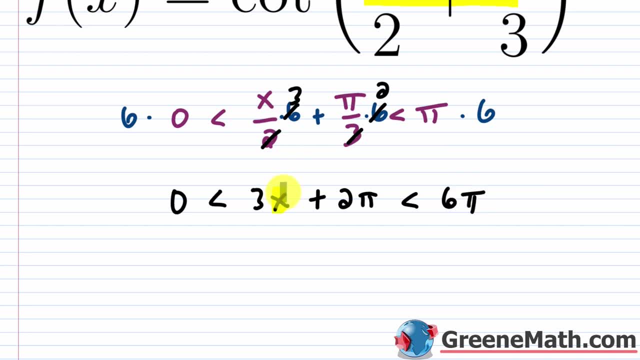 six times pi is six pi. If you want to isolate x in the middle, then what you're going to do is subtract two pi away from each part. here. Let me just put minus two pi here, And so this is going to cancel. 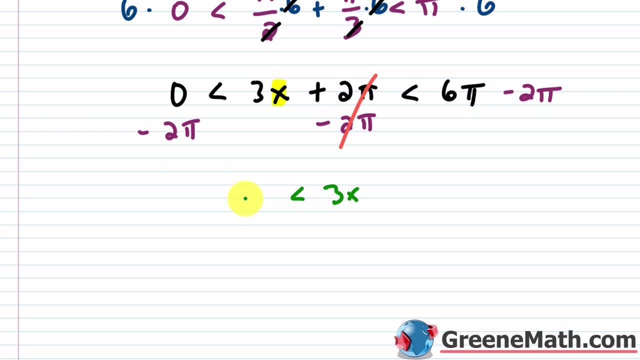 We're going to have our three x in the middle, And this is greater than negative two pi, And it's less than six pi. minus two pi would be four pi. As a final step here, let me divide each part by three, just to finish things up. So this is going to cancel, And what you're going to have is that. 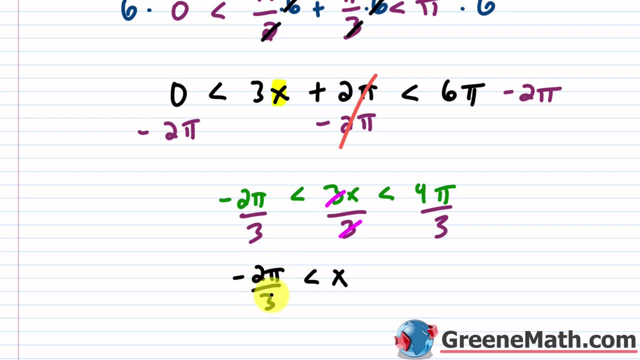 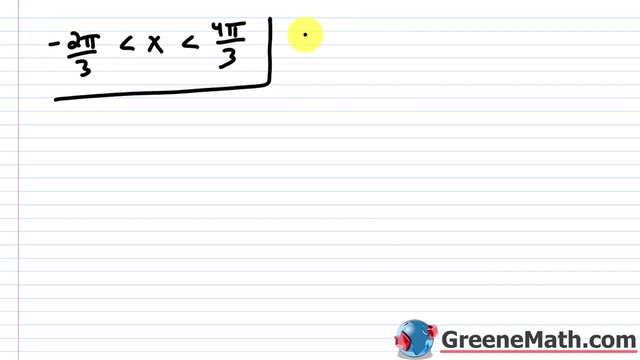 x is greater than negative two pi over three and less than four pi over three. Let me come down here and just paste this in And I'll put a little border And I'm going to say that's my consecutive asymptotes. So vertical asymptotes you're going to have: x is equal to you have this negative two pi. 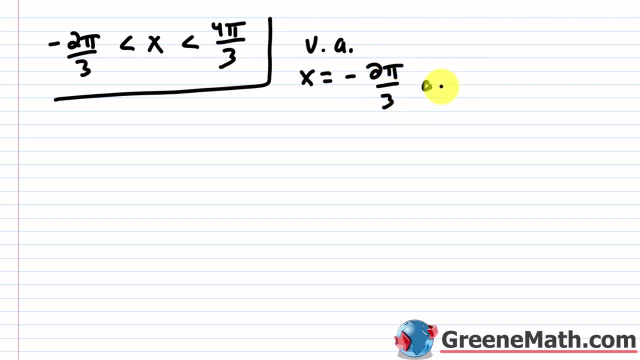 over three. And then- and let me write that better there And let me fix this- three here We're going to say x is equal to four, pi over three. Let me show you this graphically first. So, coming down to the graph, you see that you have a vertical asymptote here And this is our: x equals negative. 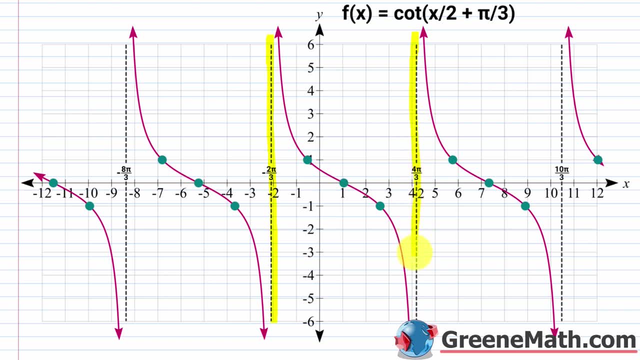 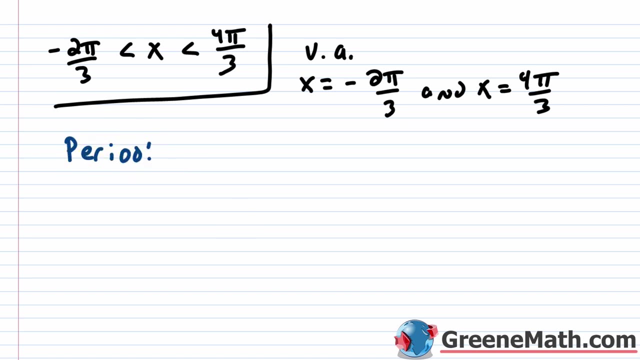 two pi over three, And then you have a vertical asymptote here. This is going to be our: x equals four pi over three, So that we know we need to figure out this point, this point and this point. So let's go back up. So what you want to do is figure out what is the period And for this, again, let's go up here. When you look at this, you have x over two, So you can think about that as one half times x. So the standard period is pi. Again, all you're going to do is go pi over one, divided by one half or times the reciprocal of that which is two over one. So this is two pi for the period. 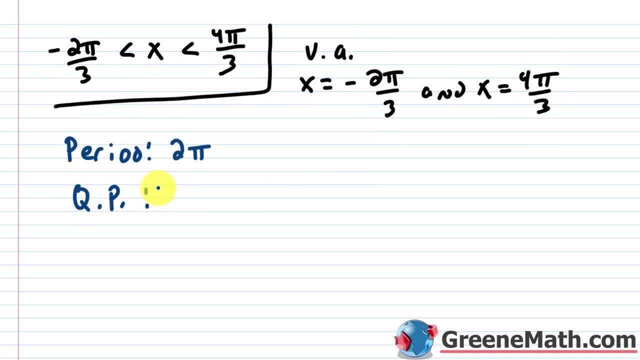 And then the quarter period: this is going to be two pi over four, which is pi over two. So again, all you have to do at this point is just go through and say: well, I'm going to go negative, two pi over three plus pi over two. So, just starting at that leftmost vertical asymptote that we found- And you need a common denominator here. So let me actually write this- I'm going to multiply by three over three. And I'm going to put this as- let me scooch this down a little bit So we have some room- This would be two pi over four. And then the quarter period: this is going to be two pi over four, which is pi over two. So again, all you have to do at this point is just go through and say: well, I'm going to go negative, two pi over three plus pi over two. So, just starting at that leftmost vertical asymptote that we found, And you need a common denominator here. So let me actually write this: I'm going to multiply. 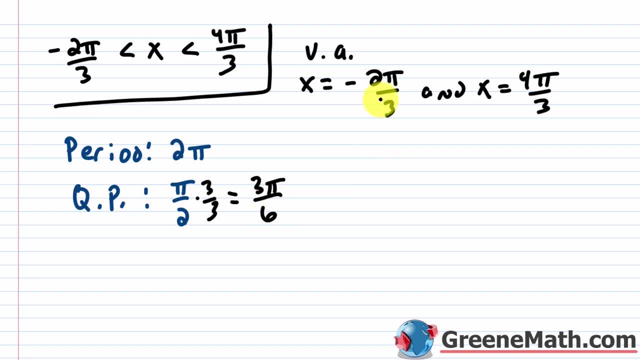 three pi over six. So I have a common denominator And this guy right here I'm going to write as negative two pi over three times two over two. So this would be negative four pi over six. So I'm just going to start with that: So negative four pi over six, and then plus the quarter period, So that's three pi over six. that's going to give you negative pi over six. So let me write this on another page For this one, your first quarter point, you're going to have negative pi over six. 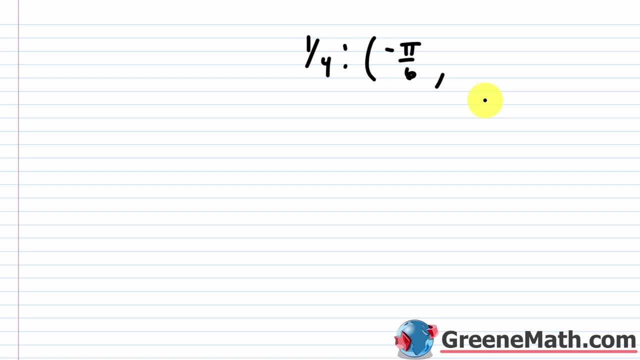 we'll get the y values in a second. I think all of you can see that there's no vertical transformations that are applied. So you could just put one now if you want, but I'll just do that separately. So then we have the one half and then we have the three quarters And let's go up and get those. So I'm going to start now with the negative pi over six And I'm just going to keep adding quarter periods. So I'm going to add three pi over six. So this gives me two pi over six, three pi minus pi. that's two pi And two pi over six. you can write that as pi over three. Let's come down here and 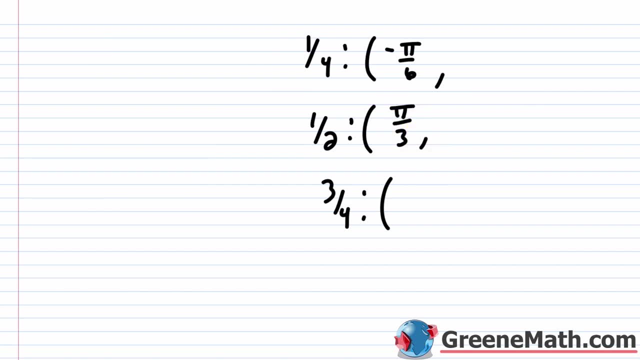 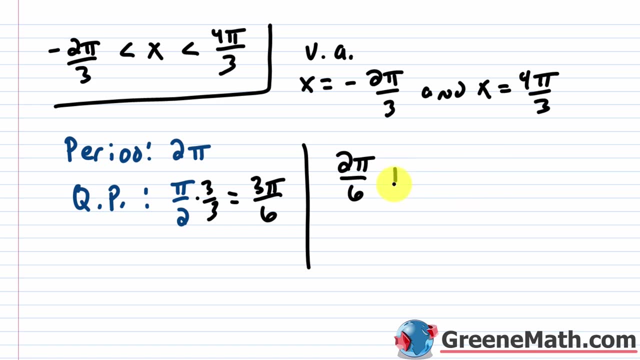 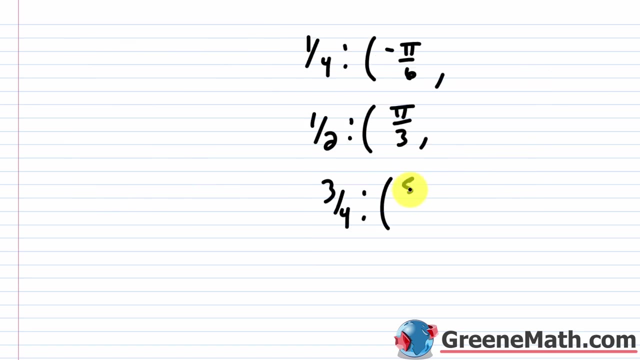 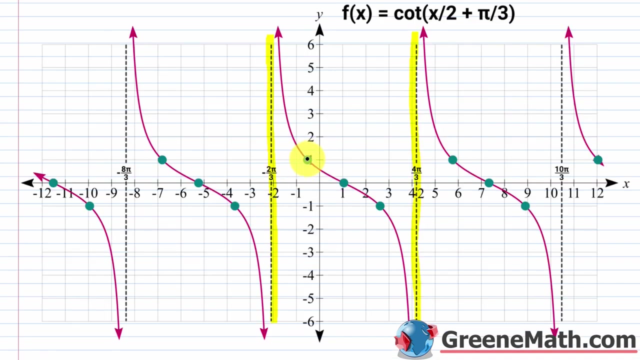 say: this is pi over three, And then let's do that one more time. So we would want to do two pi over six. So two pi over six plus the quarter period, we'll write that as three pi over six. So that gives me five pi over six. Let's come down and put five pi over six. Now for the y values. here Again, when you look at these points, you see the y value here is one, the y value here is zero, and the y value here is negative, one That perfectly matches. 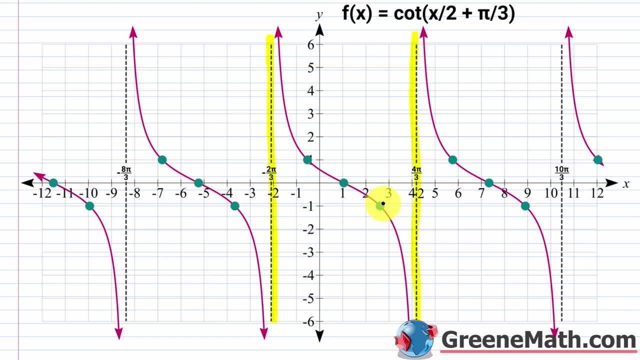 what we see with y equals the cotangent of x, And the reason for that is: you don't have any vertical transformations here. This you could really put as a one. So there's no vertical stretch or compression, And out here you don't have anything. So you can put plus zero to make. 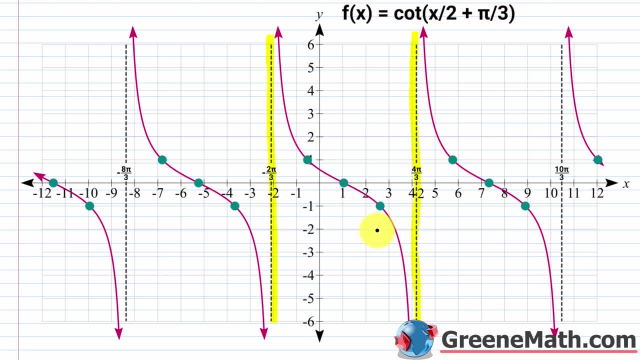 that clear. There's no shift up or down, So you would match those y values perfectly. So for the first quarter point you have a y value of one, For the midway point you have a y value of zero, And for the three quarters of the waypoint you have a y value of negative one. So let's put one. 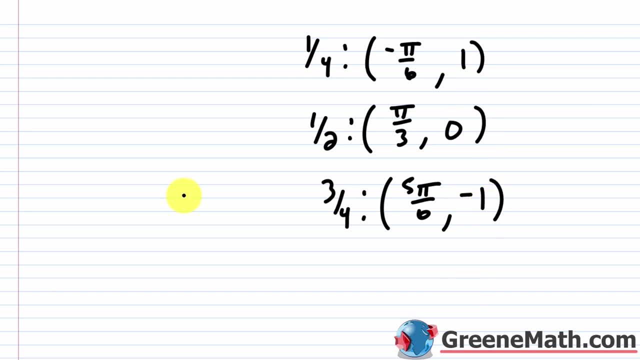 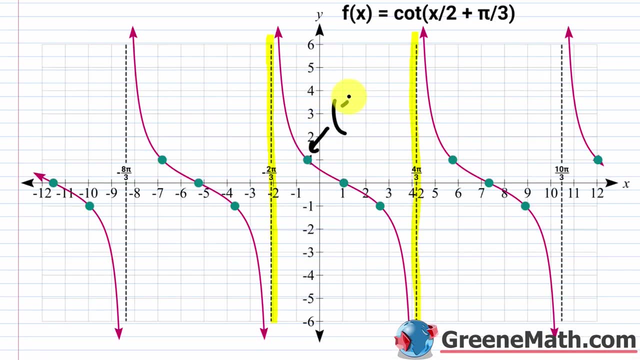 here. Let's put zero here and then negative one here. So we're ready to go in terms of labeling those points. You would have negative pi over six comma one. So that's going to be this first point right here. So this is negative pi over six comma one. That six could be a lot better And we have 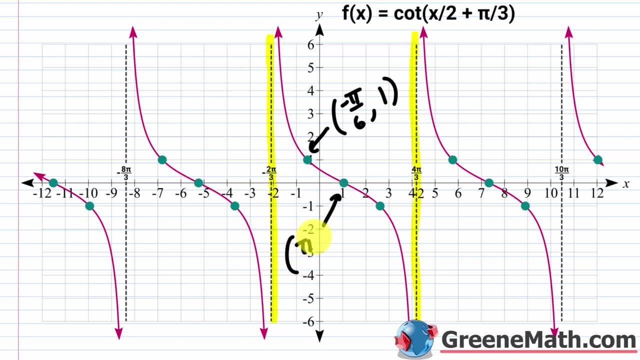 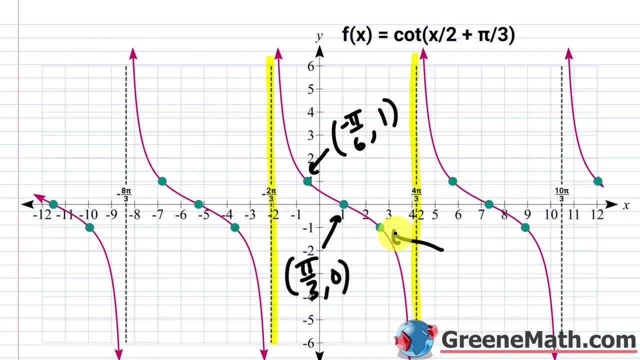 pi over three comma zero. So this one right here, let's say that's pi over three comma zero. And then this one, the three quarters of the way, it's five pi over six comma negative one. So this one will say that this is five pi over six. Let me make that six. 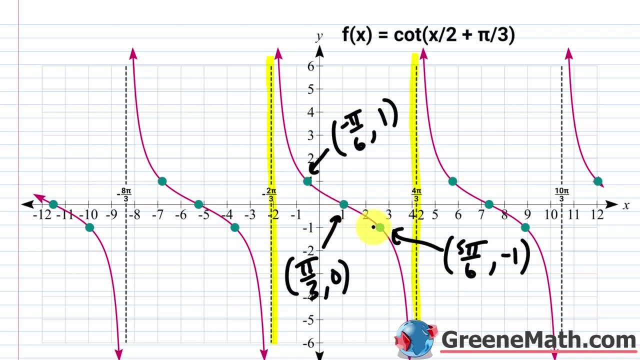 A lot better there. And then comma negative one. So those are your three key points. Again, if you want to go to the right or to the left, you just keep adding quarter periods. So in other words, if I take this five pi over six and I add a quarter period, I'm going to be at four pi over. 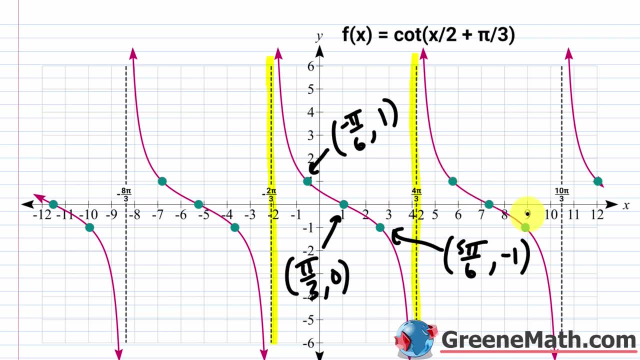 three, And you can just keep doing that to get the next point, the next point, the next point. vertical asymptote, the next point, the next point, the next point. vertical asymptote: The y values are always going to be the same, In other words, for the first quarter point. 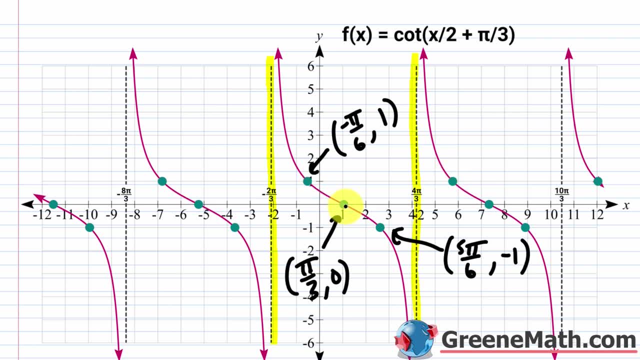 you're always going to have a y value of one. For the halfway point or the midway point, you're always going to have a y value of zero, And then, for the three quarters of the way point, you're always going to have a y value. 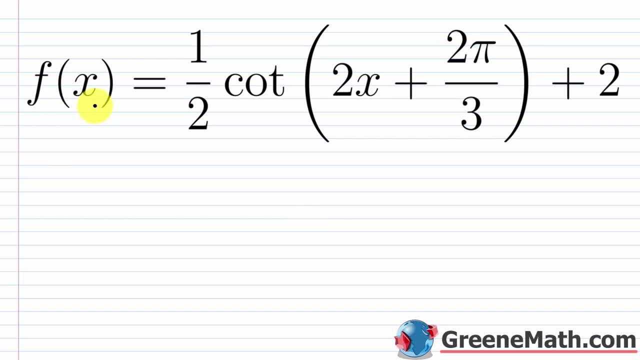 of negative one. All right, let's take a look at another one. So here we have f of x equals one half, And then cotangent of. we have two x plus two, pi over three and then plus two. All right. 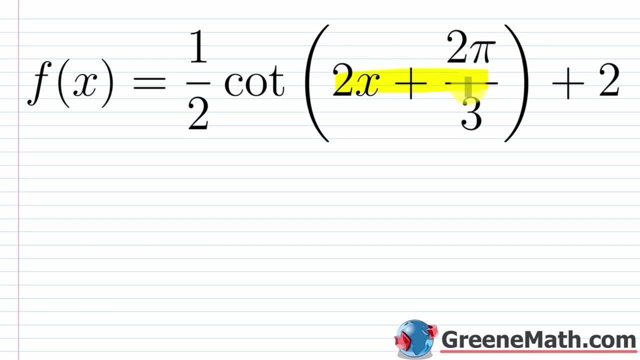 so again, I'm just going to take the inside part here. So the argument for the cotangent function- and I'm going to start by saying two x plus two pi over three is greater than zero and it's less than pi. So we'll solve this first. And so let me slide down here just a little bit. 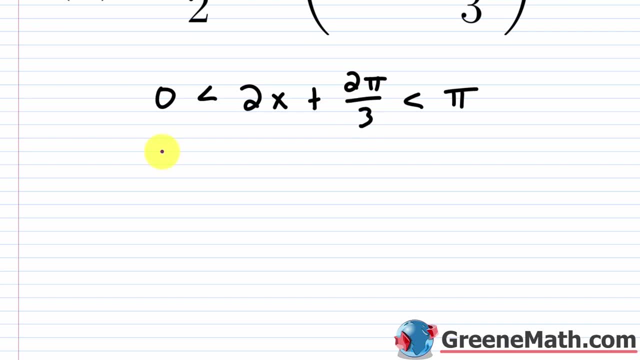 So we get rid of this denominator of three. So just multiply everything by three, So you would have zero times three. Let me show this. So zero times three is less than two x times three plus two pi over three times three, And this is going to be less than pi times three. So zero times. 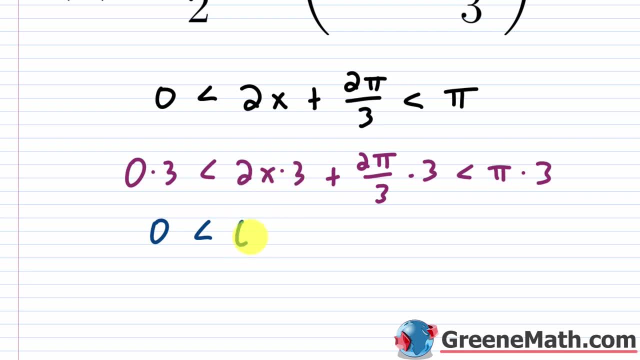 anything is zero, So this is still zero. This is less than two x times three is six x, And then plus these threes would cancel. So you have two pi. So which is less than three times pi is three pi. So at this point I'm going to subtract two pi away from each part. Let me write that down. 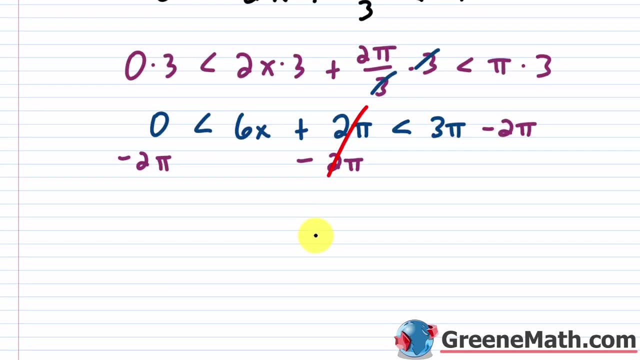 Like that, And so this is going to cancel. you're going to have six x in the middle, So this is greater than you're going to have negative two pi and less than three pi. minus two pi is pi. To finish things up, let's divide everything by six, And so that's going to give me this: 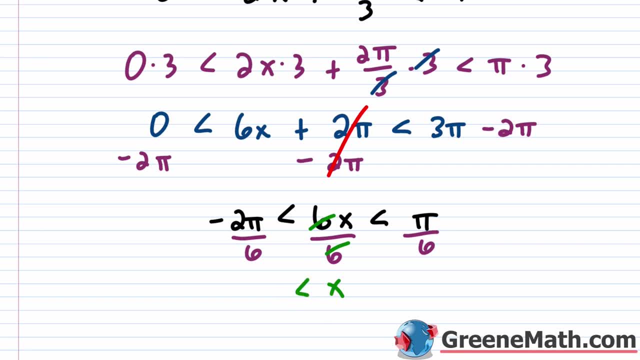 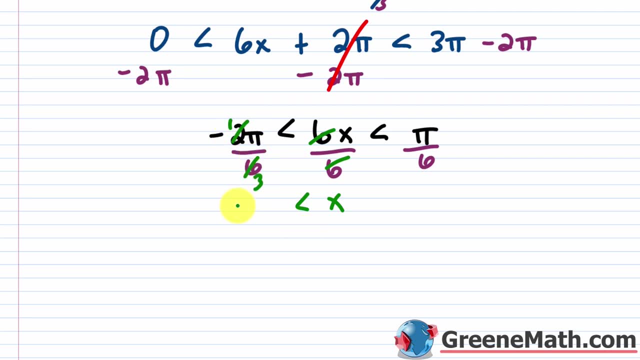 canceling in the middle. So x is greater than if you think about two and six. well, two divided by two is one and six divided by two is three. So let's say this is negative pi over three And it's less than pi over six. So let's grab this. Okay, let me put that in there like: 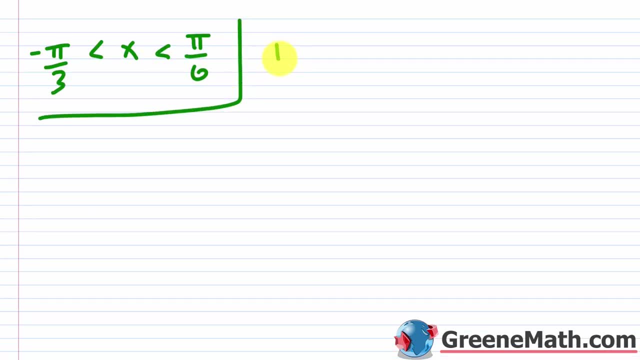 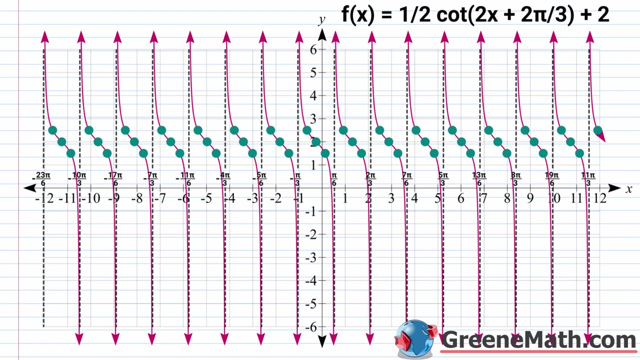 that. So again, your two consecutive vertical asymptotes. So vertical asymptotes: you're going to have x is equal to negative pi over three, And then and you're gonna have x is equal to pi over six. Alright, so this one's a little bit busy. So again, I've given you a link on Desmos, if you. 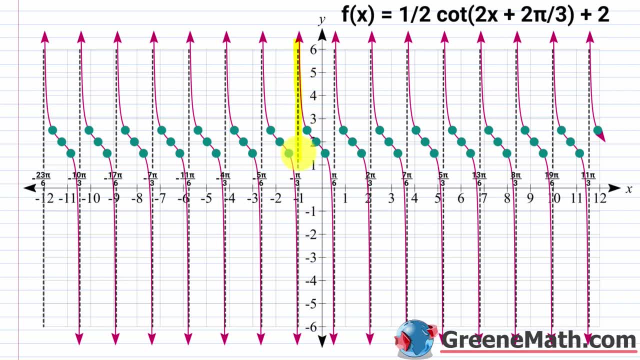 want to click that to get more detail. This is your vertical asymptote, which is going to be pi over three. So that guy right there. then this is the other one. So this is the vertical asymptote. it's x equals pi over six. So we're going to be finding these three points right here. 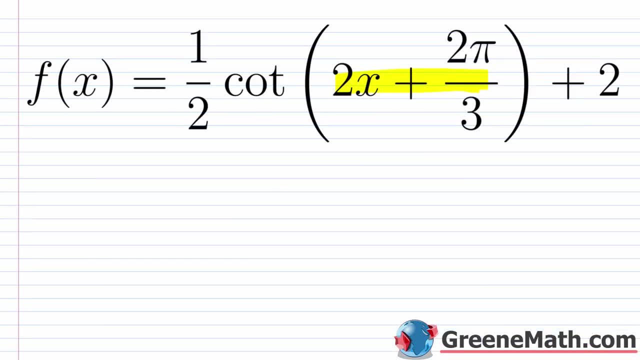 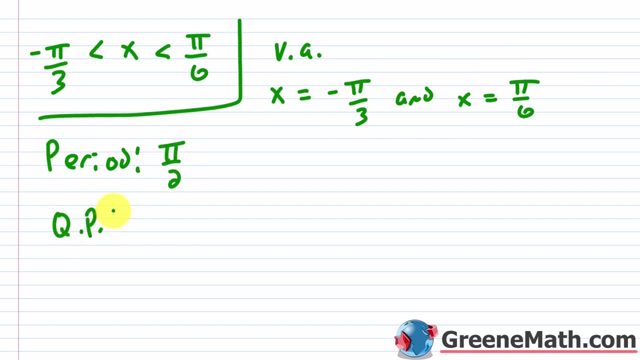 So let's go back to right here. If you want your period again, it's pi, which is your standard period, divided by two, the coefficient of x. so it'll be pi over two. So let me write that the period is going to be pi over two, and then your quarter period. So this is pi over two times a. 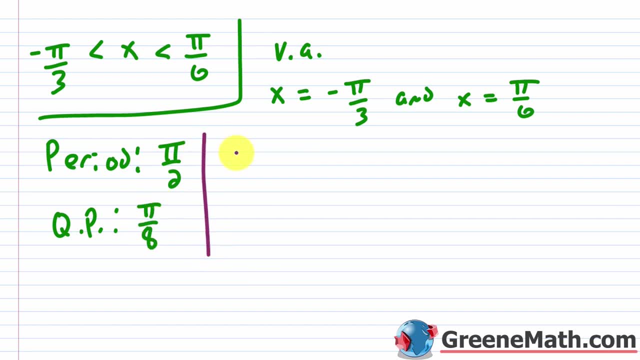 pi over eight. So again, all you have to do is take this negative pi over three and you're going to add a quarter period, So you're going to add pi over eight. Now, again, you need a common denominator. So let's just go ahead and right now multiply this by three over three, just so that. 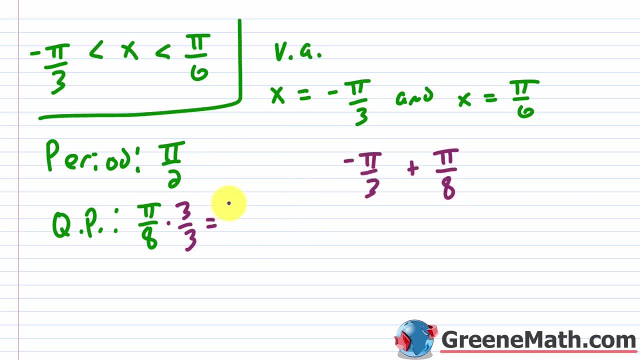 we're not struggling the whole time to get common denominators. So this right here would give me three pi over 24.. Okay, so let me adjust this. I'm going to write negative pi over three as negative eight over 24.. So then for the first quarter point the x value would be negative eight pi plus three pi. 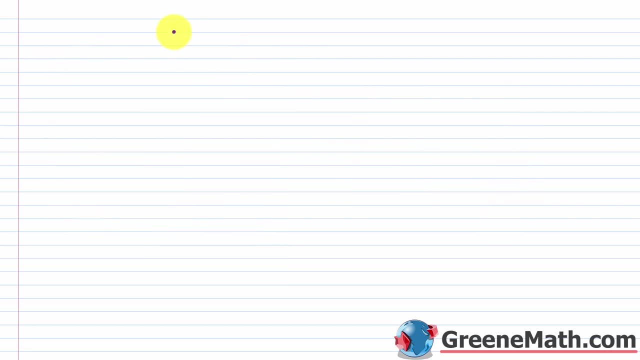 that's negative five pi and this is over 24.. And let me put for the first quarter point: you want negative five pi over 24.. Okay, so we're going to have halfway and then three quarters. we're going to figure those out right now. So let me take this negative five pi over 24.. And all I'm 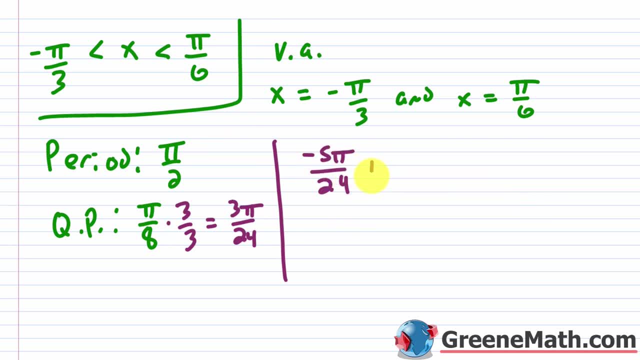 going to do is add a quarter period, So let me rewrite that it didn't take it with it. So plus four, so negative five pi. plus three pi, that's going to be negative two pi over 24.. So if you think about that, you can simplify: 24 divided by two is 12, and two divided by two is one. So this: 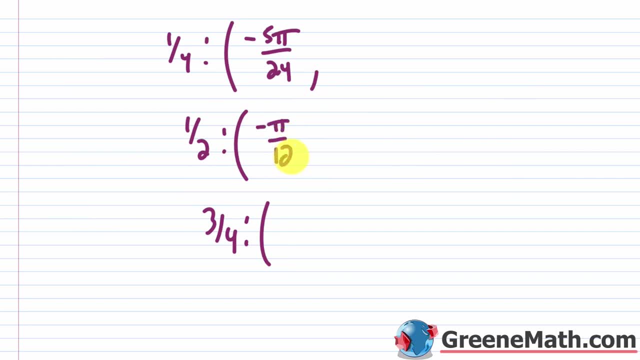 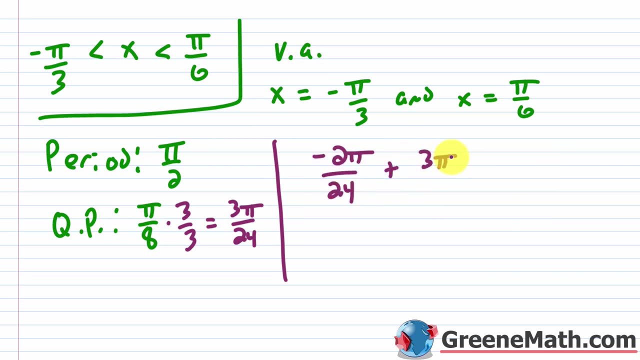 would be negative pi over 12.. So this is negative pi over 12. And let me get rid of that. And we only have one more to do, So let me move this over. So let me add three pi over 24,. one more time. 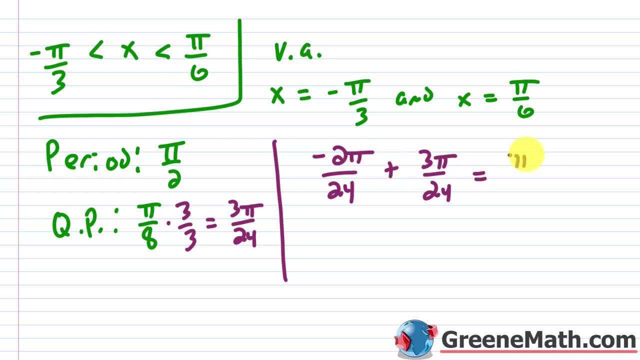 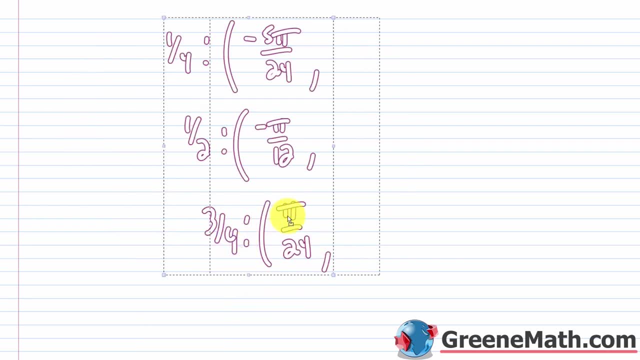 And so negative two pi plus three pi, that's going to be pi, And this is over 24.. So this would be pi over 24.. Okay, in terms of the y values, you do have to do a little bit of work here, Because you. 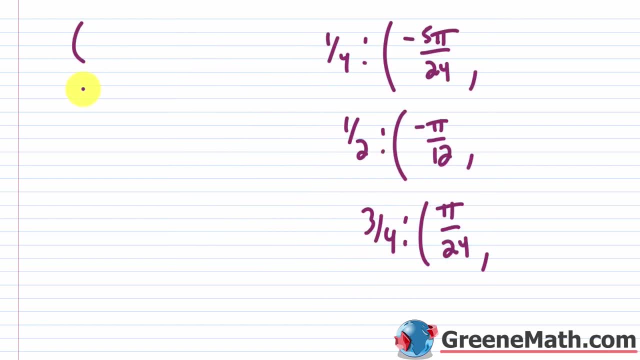 do have two transformations that are vertical. So let me start off with these basic points here. So on the y equals cotangent of x, you're going to have your pi over four comma one, then you're going to have pi over two comma zero, And then you're going to have three pi over four comma. 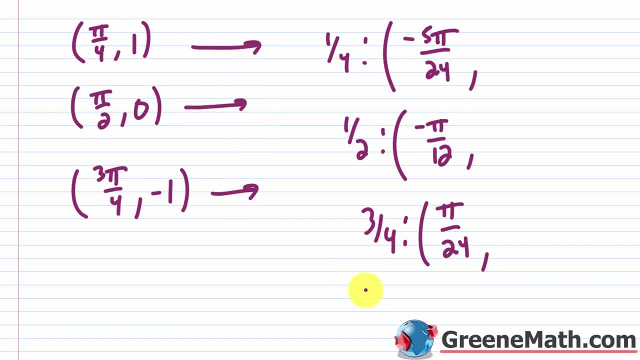 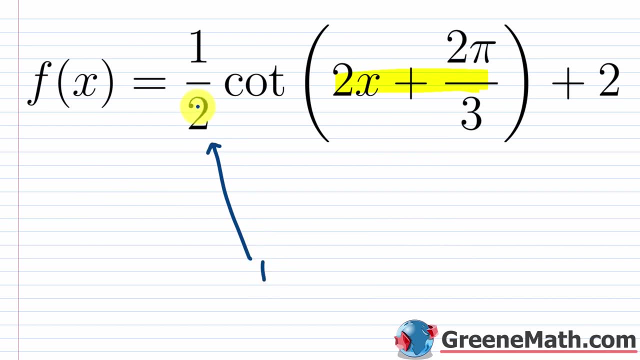 negative one. So we're going to think about how we're going to transform here. Again, in terms of vertical, you have this guy. that's done first. this is a multiplication by a half, So that's giving me, you could say, a vertical compression by a factor of two, where, again, a lot of people 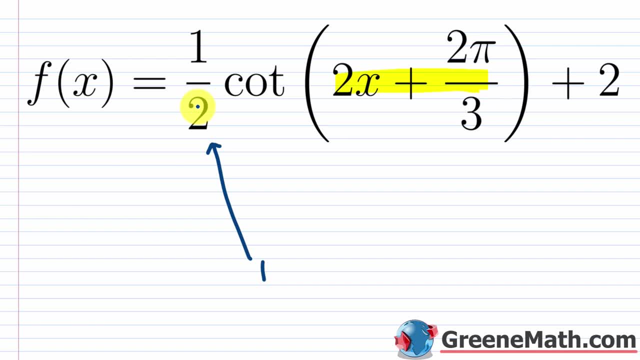 like to say it as a vertical shrink by a factor of a half. it's just understanding that you're either going to divide each y value by two or you're going to multiply by one half. it's the same thing either way, just a matter of how you want to say it. this right here, this plus two. 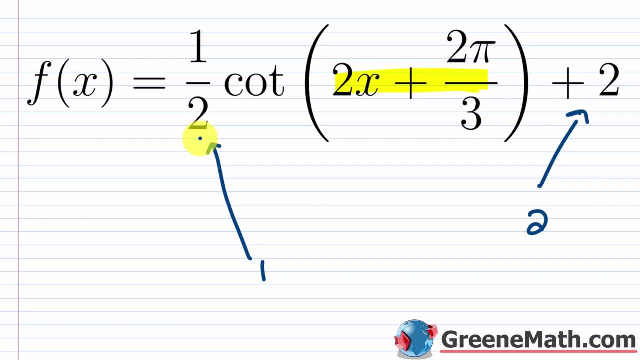 that's going to shift me up by two units. So this is done first, this is done second. So the order does matter here. So let me write this out: we're going to, for part one, multiply by one, half, or again, you could divide by two if you want, And then, for part two, we're going to add two. 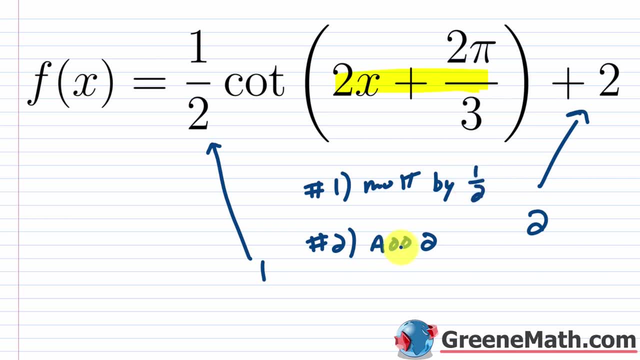 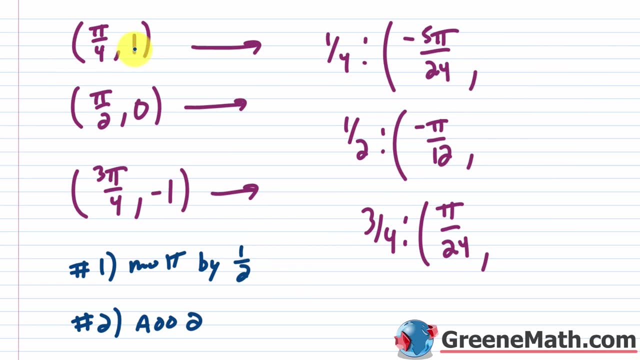 So again, this is a vertical compression by a factor of two. then you're going to add two. that's shifting me up by two units. Okay, so we're first going to multiply one by a half, So one times one half would be one half. then I'm going to add two, So you would have one half plus. 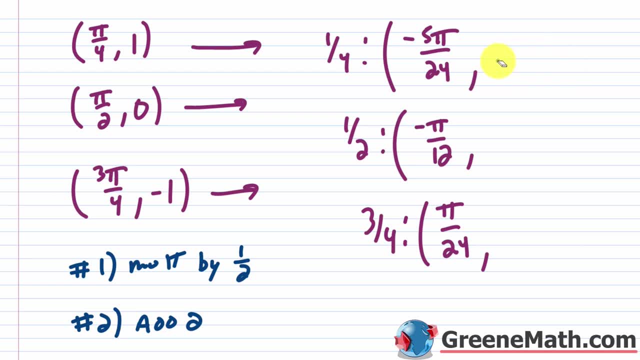 two. you could write that as four over two, So this would be five halves. So this is five halves, All right. for this one, right here, you have zero times a half. that's still zero. then you add two, that's going to be two. And then for this one, you have negative one times a half. 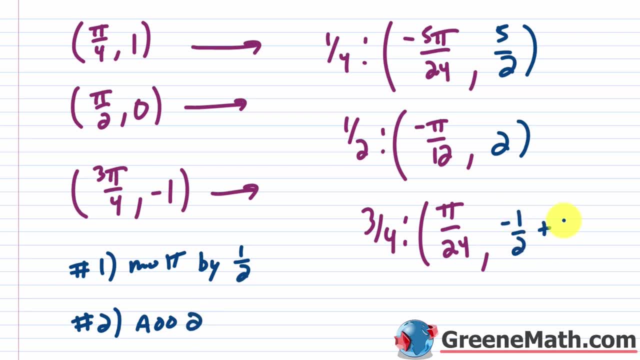 that's negative one half. and then you add two. So let's add four over two, So this would be three halves. So that's basically. it Just a matter of understanding those graphing transformations. Again, if you get confused by that, 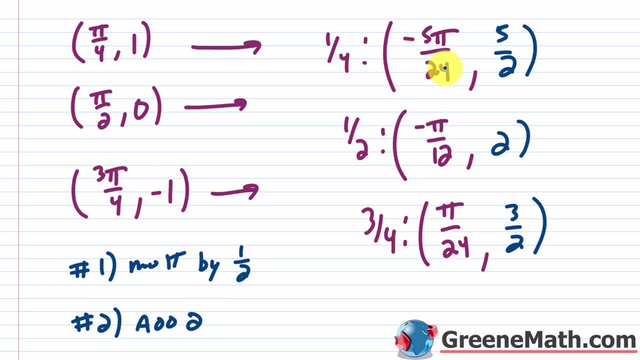 always plug in, So you could always take negative five pi over 24,, plug into the original function- you'll get five halves. you could plug in negative pi over 12, you'll get two. you could plug in pi over 24,, you'll get three halves. All right, let me get rid of this And let's just label things. 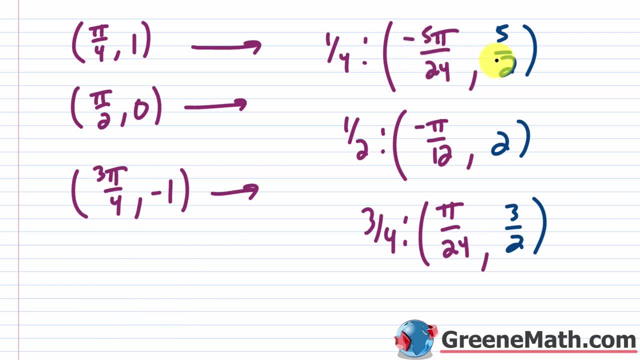 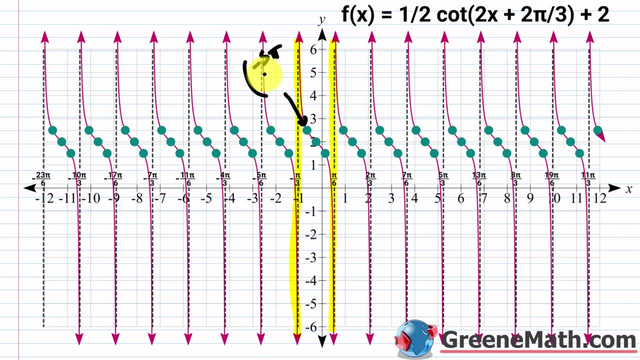 and we'll be done So for this one right here you have negative five pi over 24 comma five halves. So that's going to be this one right here. So this is negative five pi over 24 comma five halves And if you look at this it's hard to see. but this notch right here is two. 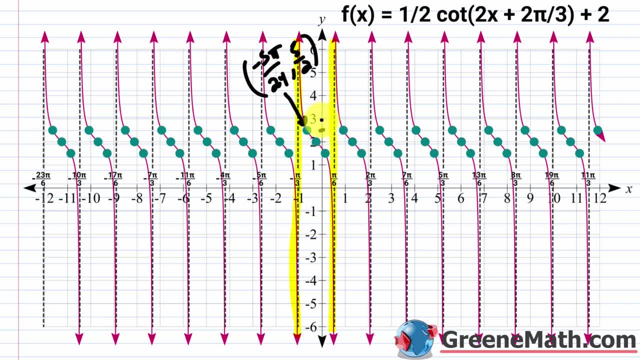 so this notch right here would be 2.5, because this notch right here is three. And then if you look at this one right here, that's going to be negative pi over 12 comma two. So that is negative pi over 12 comma two And again, this notch right here is two. it's covered up by that point And 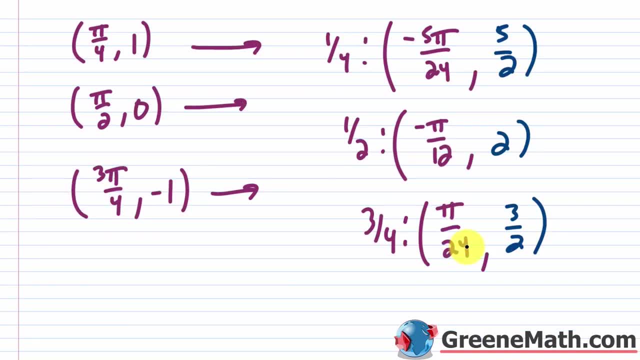 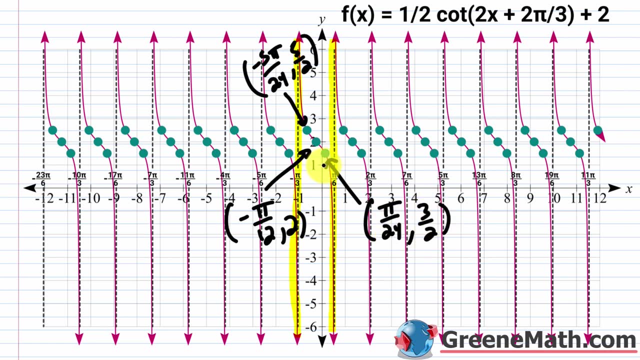 then if you look at this one right here, we're going to have pi over 24 comma three halves. So this is pi over 24 comma three halves. And again, this notch right here is one, this notch is two. So this is halfway. So that's 1.5 or three halves in terms of your 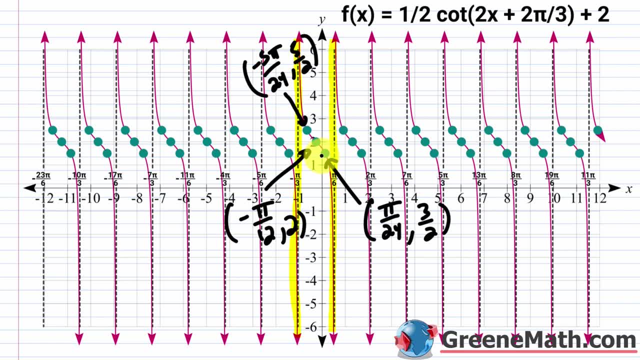 y value. So you can see that does match up. Again, if you want to click the link on Desmos, you can see I've labeled all of these points for you So you can go through there and you can get some additional practice by basically just adding quarter periods to this guy, So to the x values. 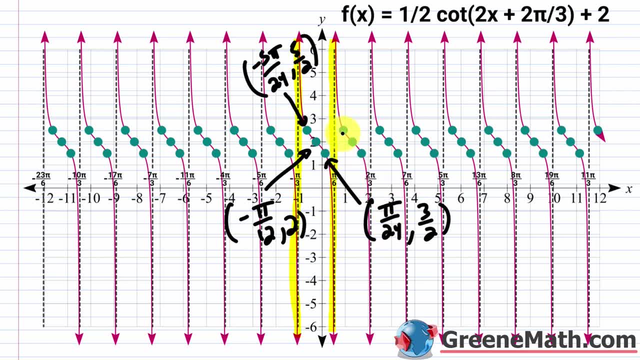 here you'll get your vertical asymptote, And then you're going to get the x coordinates for this guy, this guy, this guy- vertical asymptote. this guy, this guy, this guy- vertical asymptote, so on and so forth. You know the y values are always going to be the same. So for the first, 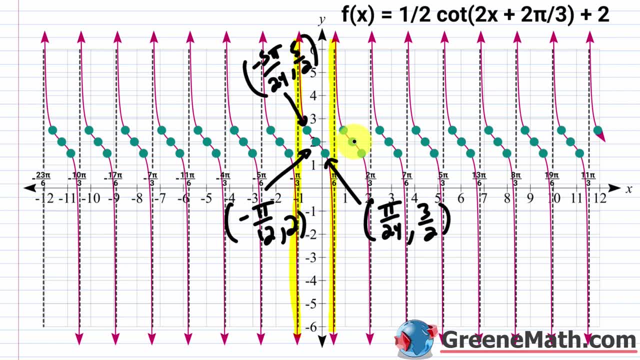 quarter point, you're going to have five halves. Then for the midway point you're going to have two, Then for the three quarters of the way point you're going to have three halves, so on and so forth. So if you want to play around with it and get some additional points going on, 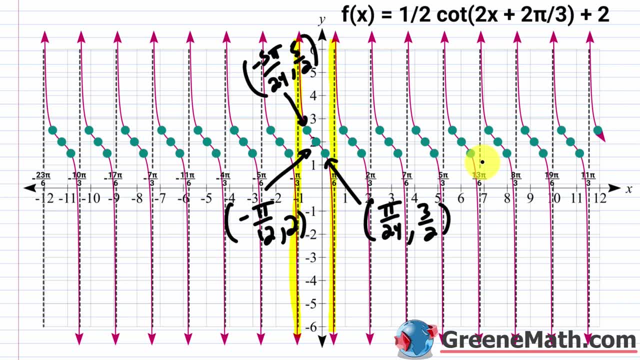 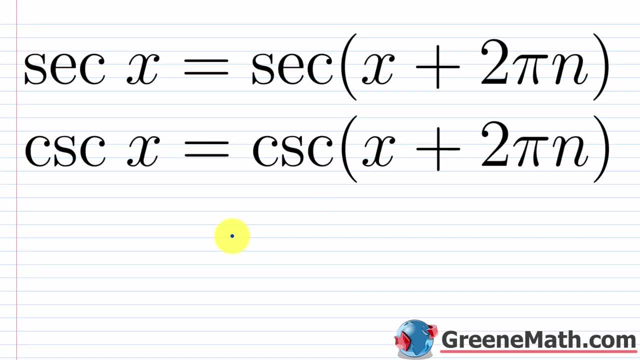 your graph going to the right and to the left. it'll be good to get some practice. In this lesson we want to learn about graphing secant and cosecant. All right, before we get started with the lesson, I want to remind you that when you're in this section, 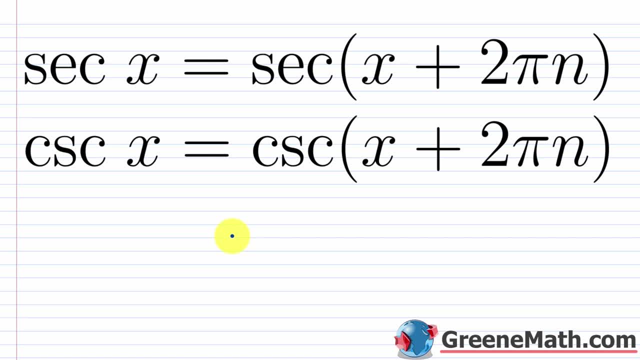 and you're graphing trigonometric functions. we want to understand the concept. So how could I graph the function if I wanted to? But generally speaking, if we want to get a perfect graph, we're going to use graphing software And that's something we're going to rely on as we get out of. 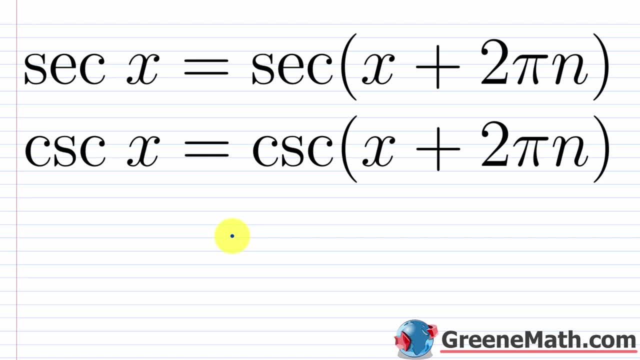 this chapter. So don't worry too much about trying to make some perfect graph, just do the best that you can. So when we look at this, we're going to start out by saying that in our lesson on cosine and sine, we learned that the period was two pi When we think about something like the secant. 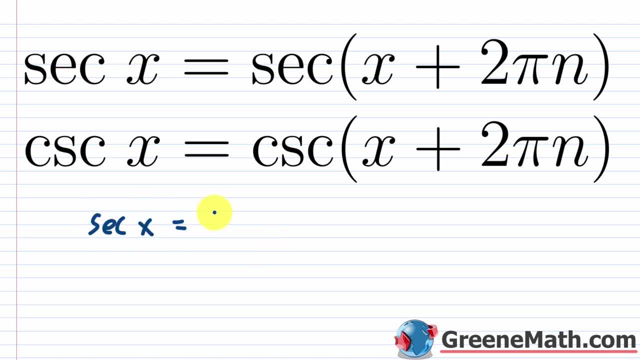 function. so the secant of x, this is equal to one over the cosine of x. So what would the period for the secant function be? Well, it's going to be two pi as well. The secant of x is equal to. 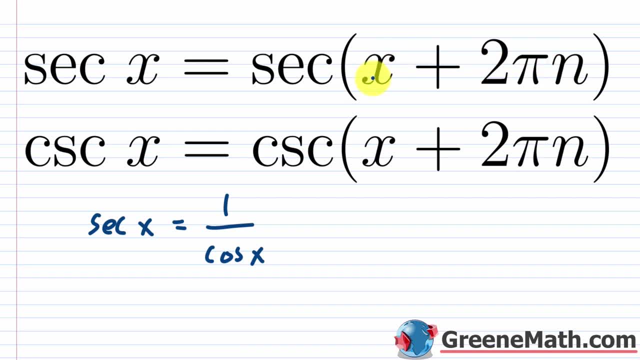 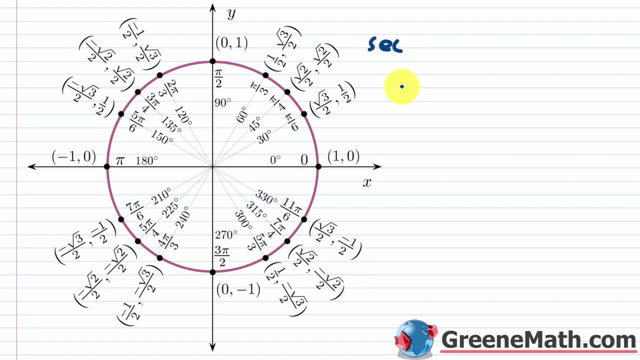 the secant of you have this x plus two pi n, where x is a member of the domain and n is any integer. In other words, if I was to come to the unit circle and let's say that I took the secant, 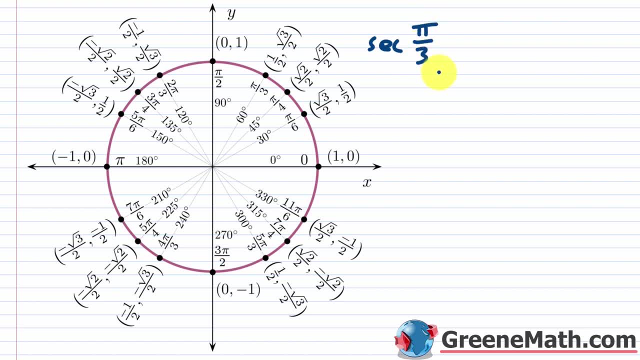 of. let's just do pi over three, that's an easy one. So the secant of pi over three, this would be equal to, by definition, one over the cosine of pi over three, And so the cosine value for this pi over three. again, you just look at the x coordinate, so that's one half. So this would 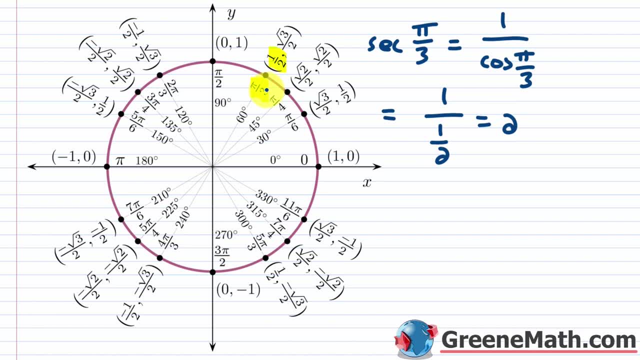 be equal to one over one half, which would be two. If you added integer multiple, you would have two multiples of two pi to this angle: pi over three. So in other words, you could add two pi to it, four pi, six pi, or you could subtract away two pi. subtract away four pi something. 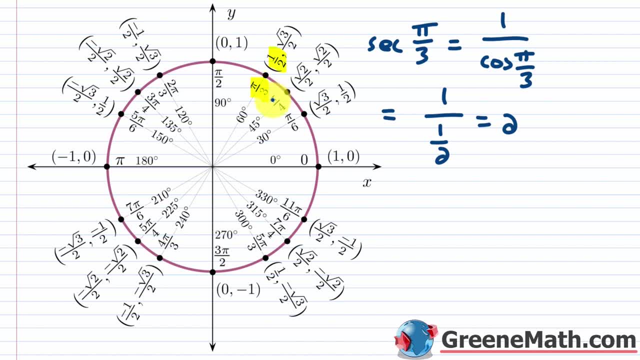 like that. You're going to end up with a coterminal angle, So you're going to have the same cosine value and also the same secant value. So just to keep it simple, let's say we have the secant of 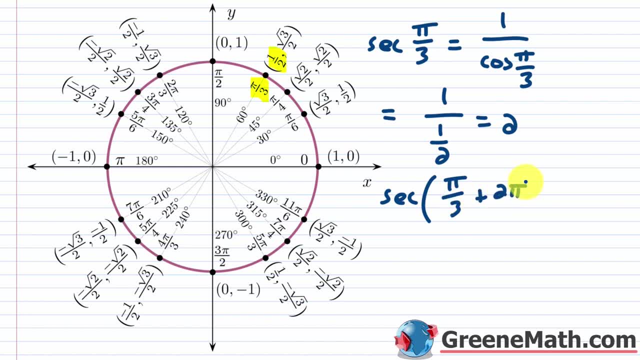 let's go pi over three plus two pi, And I would write that two pi as six pi over three. So we have a common denominator, So six pi over three. So this would be the secant of seven pi over three, And of course that's going to be coterminal with pi over three. So we know that. 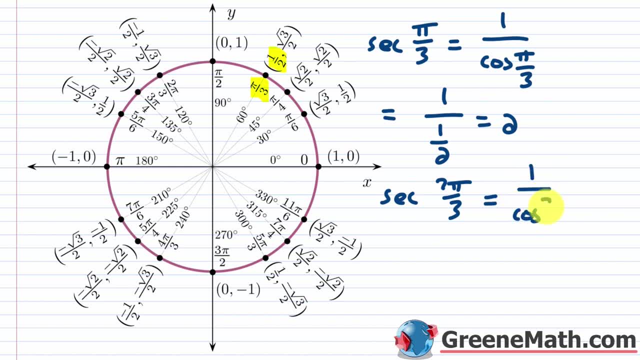 the cosine value would be the same. So this is one over the cosine of seven, pi over three, which would be equal to again one over this one half, which would be two. So the period for secant is going to be two pi. Now let's talk about cosecant. So, using a similar thought process, 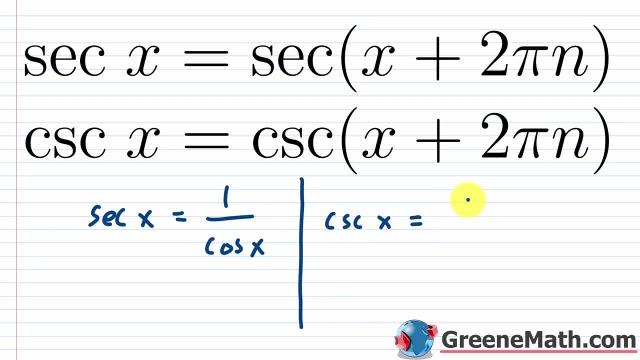 when we think about the cosecant of x, this is equal to one over the sine of x, And of course sine function is two pi, So the period for the cosecant function would be two pi as well. So the cosecant of x is equal to the cosecant of x plus two pi n, where x is a member of the domain, and n. 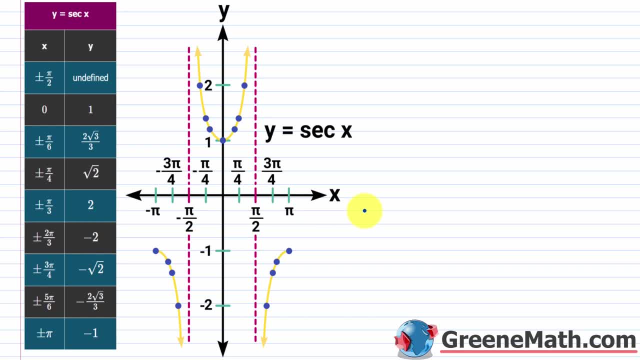 is any integer, All right. so we're going to start out by looking at the secant function And we're going to do that with a table of values And we're going to look at this over one period. So y equals the secant of x. we're going to say, where x is greater than or equal to negative pi and less. 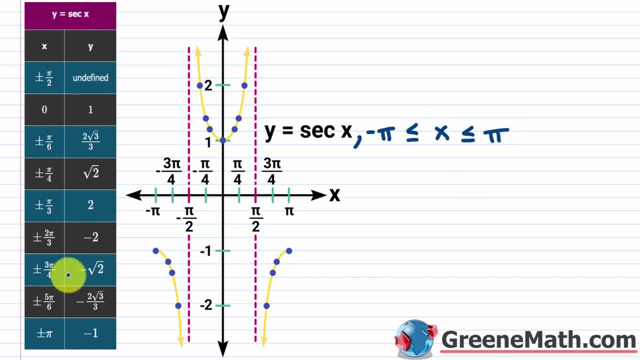 than or equal to pi. Now we're not going to use this table of values approach when we graph secant. in general we'll have a different procedure for that. We're just using this to get some key points here Now with the other graphs for sine and cosine and then also with tangent cotangent. 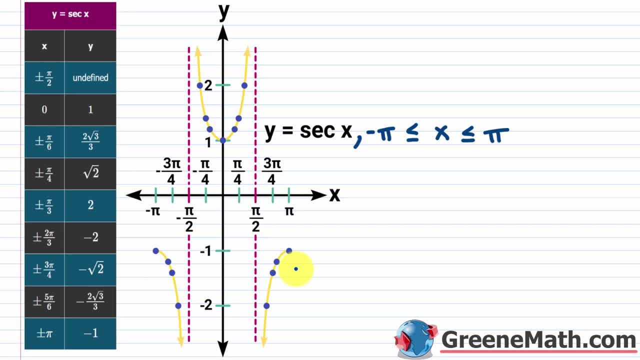 there were points that you really needed to memorize. you're not going to do that here, because you're going to end up using the cosine function as a guide, And we'll get to that later on, For right now, I'm just going to focus on some things that we want to know, And so the first 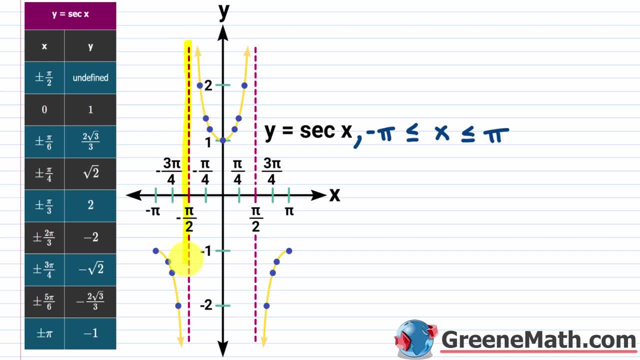 thing would be that you have a vertical asymptote here at negative pi over two and then also at pi over two. So we want to think about where that comes from. Remember that the secant function of x is equal to one over the cosine of x. So just like we saw with a tangent function, 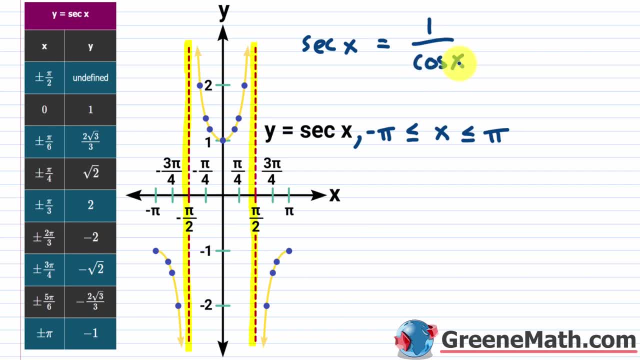 you have your cosine function in the denominator there. So wherever the cosine values are zero, you're going to get division by zero, which is undefined, And that's giving you these vertical asymptotes. So that's going to happen at odd multiples of pi over two. So negative pi over two. 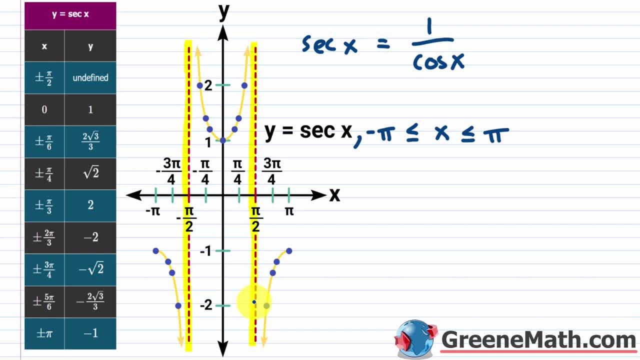 pi over two, three pi over two, five pi over two, so on and so forth. Now, another thing I want to call your attention to is that when you look at the behavior of this graph, so let's say as this example to an x value of pi over two, Now it's not actually going to get to an x value of pi over. 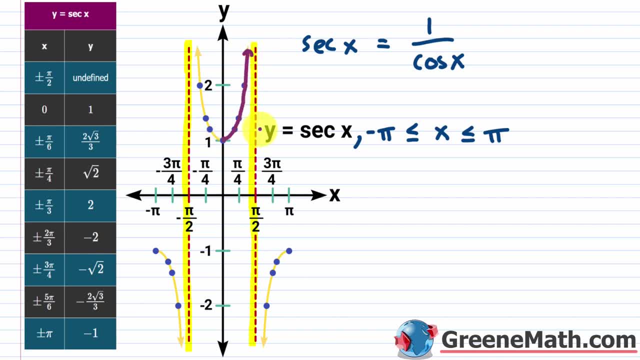 two. but you want to think about what's happening as it approaches an x value of pi over two coming from the left. So we would think about something like: let's say secant of, let's just do pi over three again. that's an easy one. This is equal to one over the cosine of pi over three, which is one. 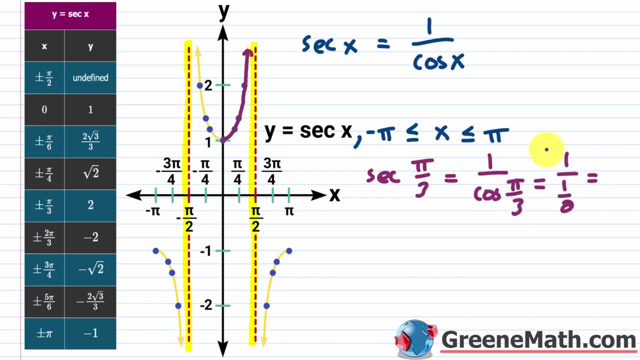 over again. the cosine of pi over three is a half. So notice that this value right here of one. when I divide by a half, I get something bigger. I get two. When you take one and you divide by, you're going to get something that's larger than one. For example, if I did, let's say, one divided. 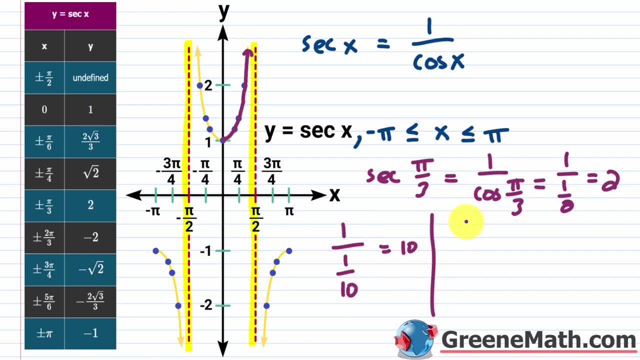 by one 10th, I would get 10.. Or let's say, as another example, I did one divided by one over 100. Well, that would be 100.. So what's going to happen is, as the x value here gets closer and 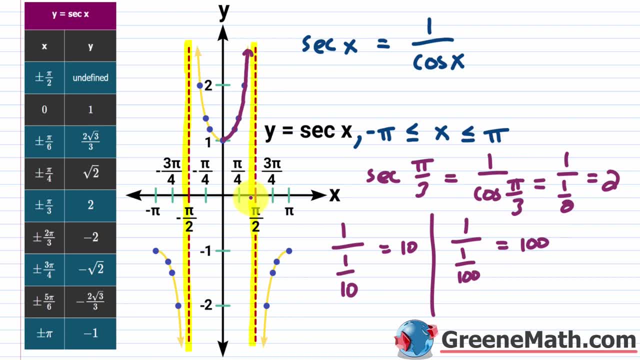 closer to pi over two, the cosine value gets closer and closer to zero. So you can get as close to zero as you'd like, but you can't actually touch it. So what's happening is the value is going to get really large for secant because you have that one divided by that number. 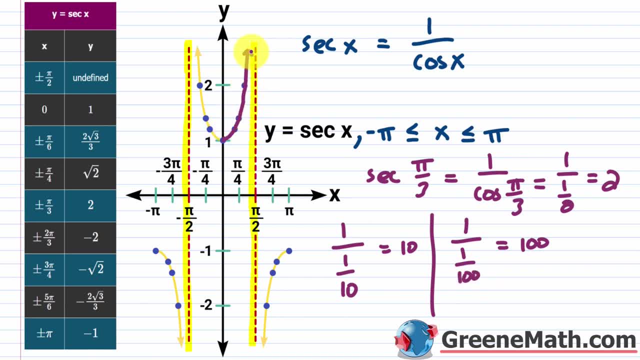 that's really really close to zero. So this guy right here is going to priest without bound or, as they say, approach positive infinity. So let me get rid of this. And we also want to think about the other side of that. So at pi. so the secant of pi is equal to: 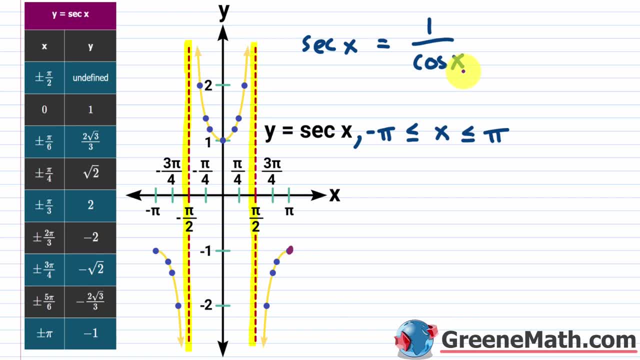 one over the cosine of pi. So we know that the cosine of pi is negative one. one over negative one would be negative one. So here this point would be: pi comma, negative one. Now what happens as we approach pi over two coming from the right? In other words, what's going on right here? 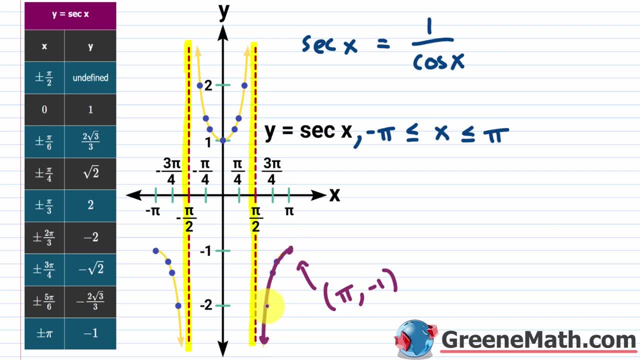 and you'd see that we're decreasing without bound, So we're approaching negative infinity. Basically, what's happening is if you think about something like, let's say, the secant of two, pi over three, to make it simple, So there's a pi over three. reference angle: 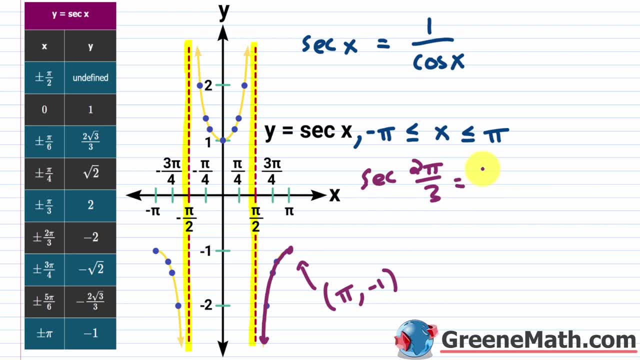 So we know that we're in quadrant. two cosine is negative, So this would be one over the cosine of two, pi over three, and this equals one over. now you'd have negative one half, And so this would be negative two. So it's the same thing here. If you look at that point, it's going to be right. 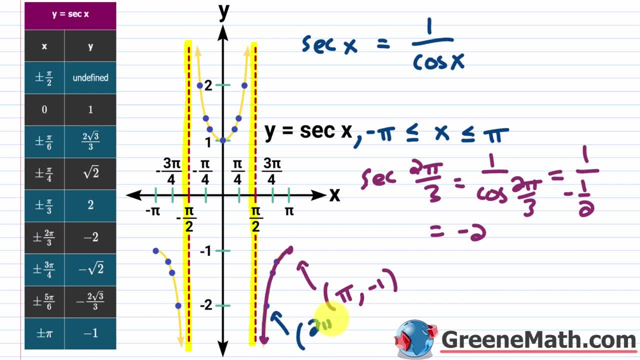 there. So this would be your point, which would be two pi over three, comma negative two Again, as this x value gets closer and closer to pi over two. again, coming from the right now, the cosine value is getting closer and closer to zero. 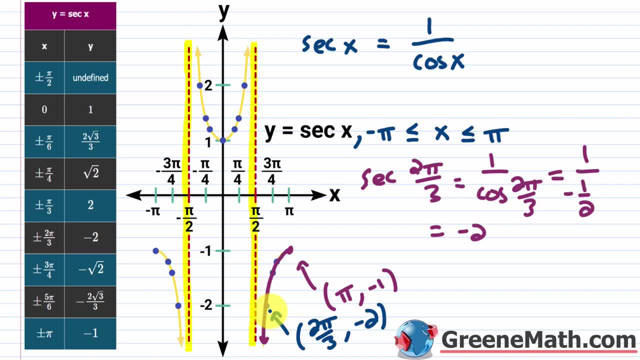 but it's on the other side of zero, So it's going to be something between zero and negative one now. So this guy is now going to approach negative infinity. So that's just something you really need to understand about the behavior of this graph. That's why 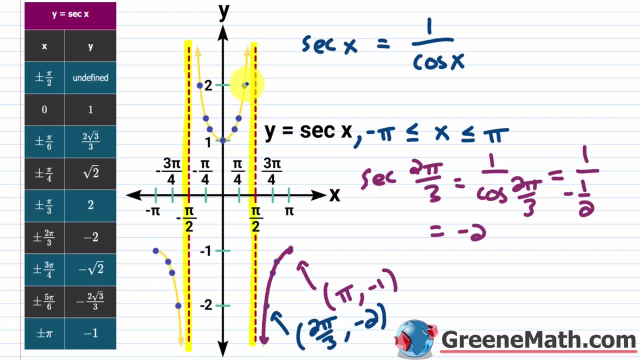 you have this going this way. That's why you have this going this way And that's why you have this shape right here. So once you understand that, it's basically good to go into the next step. So let's go ahead and do that. So let's go ahead and do that. So let's go ahead and do that. 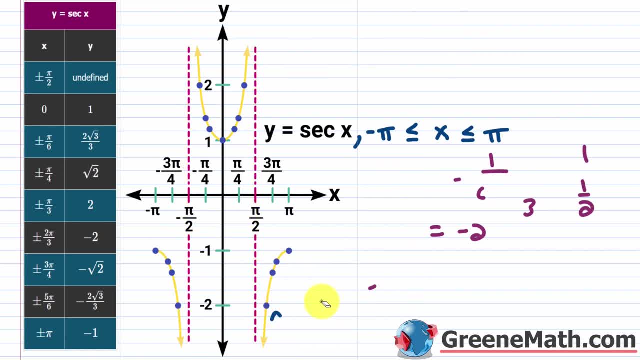 Why the graph looks the way that it does. And now what I want to do is just erase some things and give ourselves a little clean slate here, And I want to go through some of these basic points. So, first off, you should know this point right here, which is zero comma one, That's one, that's. 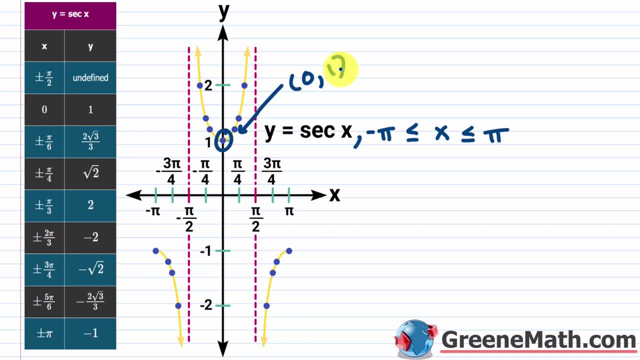 going to be on the graph of your cosine function and your secant function. Then this one right here: this is your pi comma negative one Again. that's going to be on both. And then this one right here, that's going to be negative pi comma, negative one. Now, in terms of these other points, 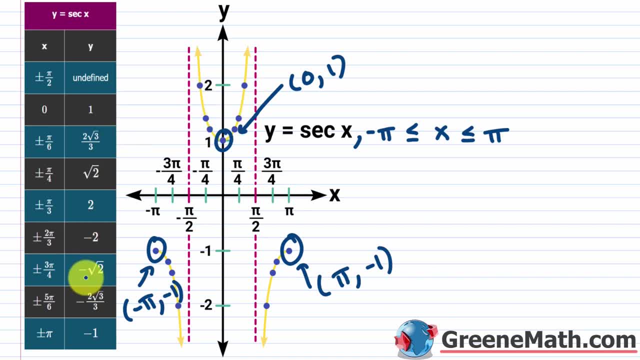 if you want to go through them in more detail, I left you a link on Desmos So you can stop the video here. click that link and you can look at all these points and think about where they're coming from. I'll just read through them real quick, If you have. 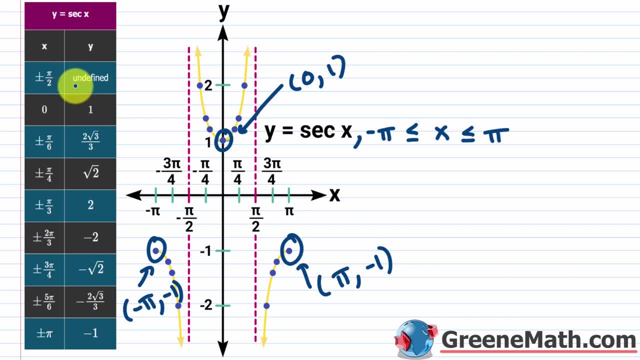 plus or minus pi over two. again. that's where we're going to be undefined, because the cosine value is zero. You have zero comma one. So that's this point right here. Then this plus or minus pi over six, you get two times square root of three over three. Let me actually show you that real. 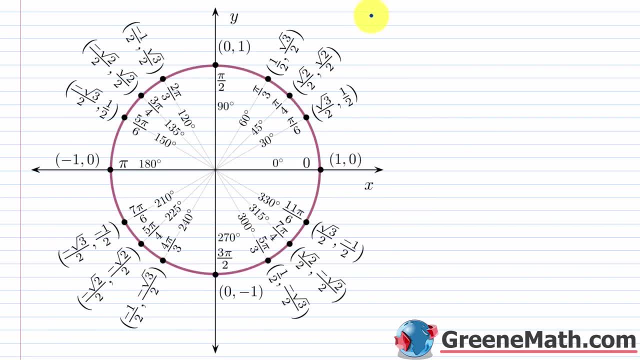 quick, So these other guys make sense. Coming back to the unit circle Again, if I asked you for the secant of pi over six or I asked you for the secant of negative pi over six, you're going to get the same thing because 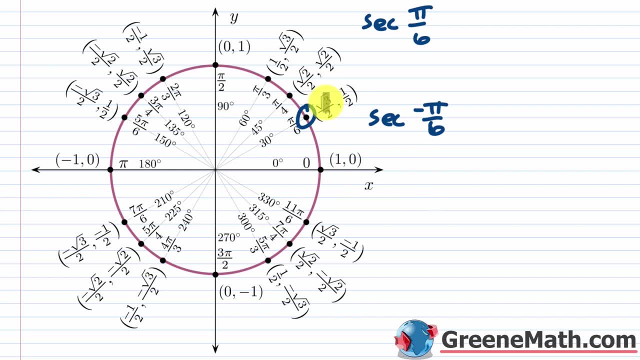 again, when you look at pi over six, the cosine value is square root of three over two. When I look at negative pi over six, again, that's rotating clockwise. So that's coterminal with 11 pi over six. Let me write out that this is negative pi over six here, So the cosine value 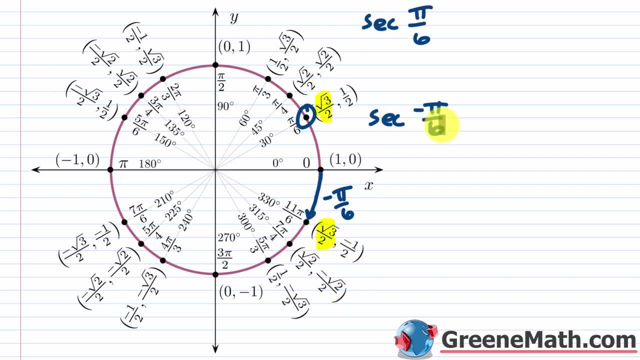 is again square root of three over two. So whether I take the secant of pi over six or the secant of negative pi over six, again, I'm going to be in either quadrant one or quadrant four, where cosine and secant are positive and I have the same reference angle. So I'm going to get the 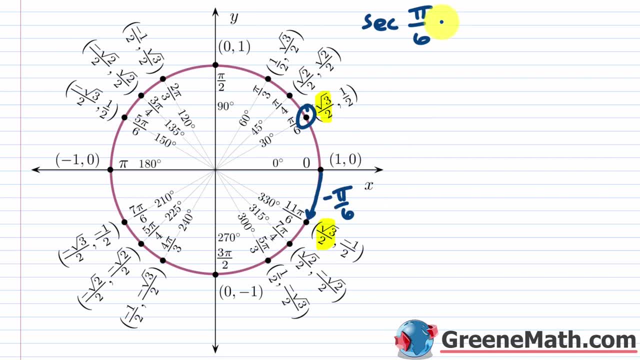 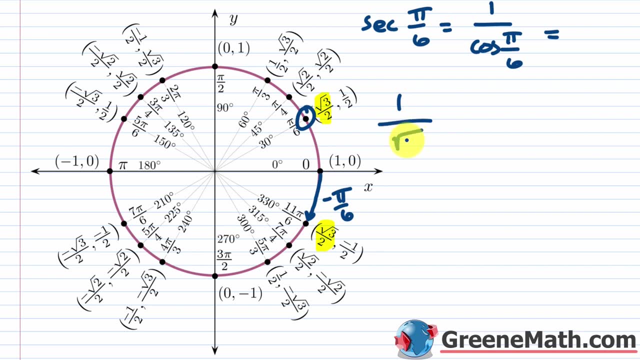 same result. Let me just do this one real quick. You can get rid of this one. I'll just show you this real quick. So this would be equal to negative pi over six. So I'm going to get the one over the cosine of pi over six And of course, this is one over the square root of three. 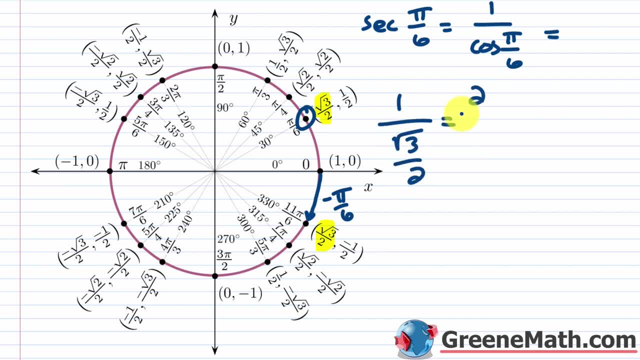 over two, And so this would be equal to. you're just going to flip this and say this is two over the square root of three and then multiply it by the square root of three over the square root of three to rationalize the denominator. So you get two times the square root of three over three. 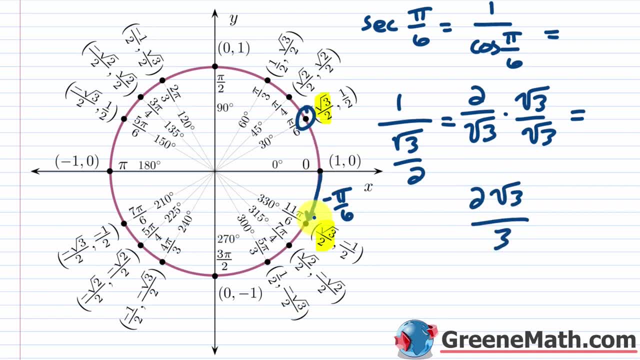 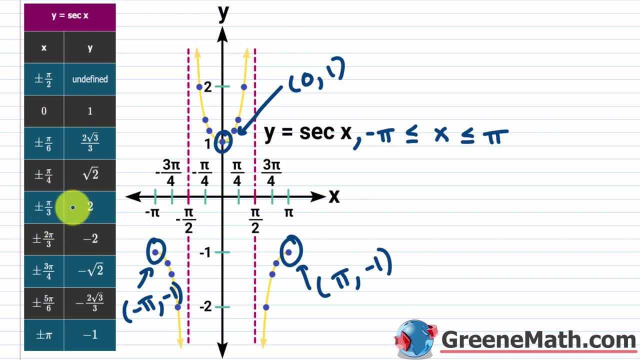 And again this would be for pi over six or negative pi over six. So, coming back down again, plus or minus pi over six, you're going to get two times square root of three over three. Plus or minus pi over four. you're going to get square root of two Plus or minus pi over three. 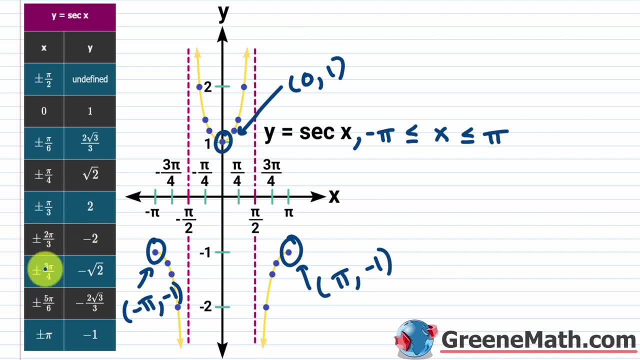 you're going to get two Plus or minus two. pi over three you're going to get negative two Plus or minus three. pi over four you're going to get negative square root of two, And then plus or minus five pi over six, you're going to get negative two times square root of. 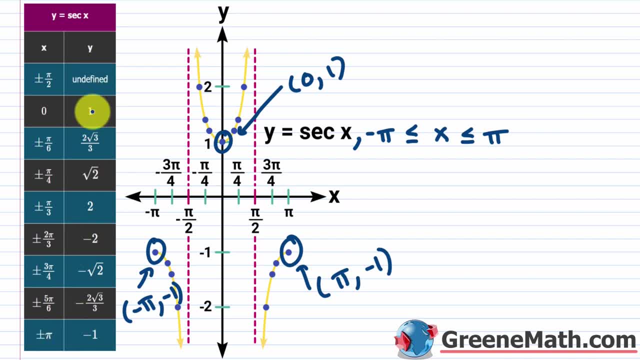 three over three And then plus or minus pi, you're going to get negative one. You can look at that link again on Desmos if you want to go through those points Again. we're not going to focus too much on these points. We're going to use the cosine function as a guide, So don't worry. 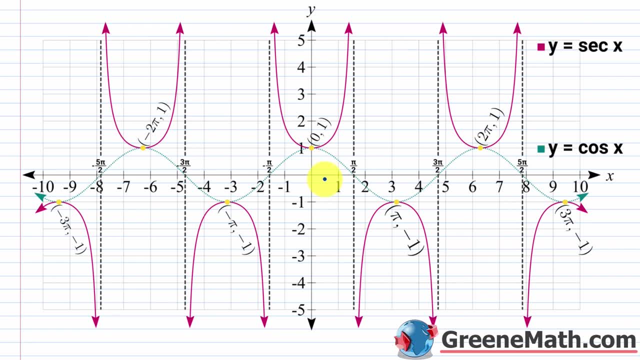 about this too much. Okay, now let's actually get into the procedure. So how do you sketch the graph of the secant function? Well, you're going to use the cosine function as a guide. So you know how to graph the cosine function at this point. If you do it over one cycle, you would do this part. 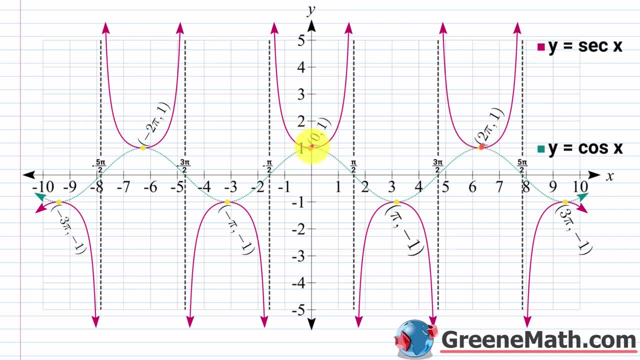 right here And I'm just going to trace over this real quick. So from zero to two pi. So this is what your basic cosine function looks like, And we've graphed that a million times at this point, So you would graph that guy right there, And then what you're going to notice is that you have a 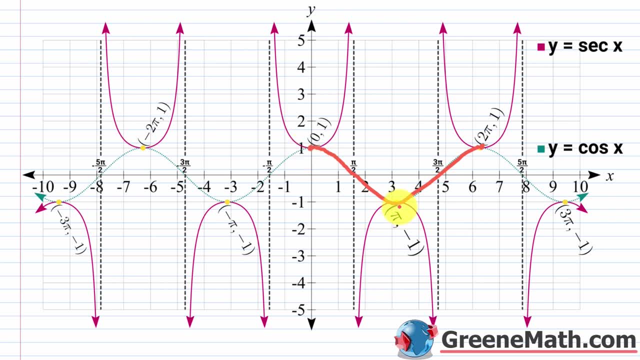 shared point here, So at zero comma one, and then also here at pi comma negative one, and then also at two pi comma one, And I'll talk about how those come into play in a moment. But you'll notice that where you have an x intercept, So that's right here at pi over two and right here at three pi. 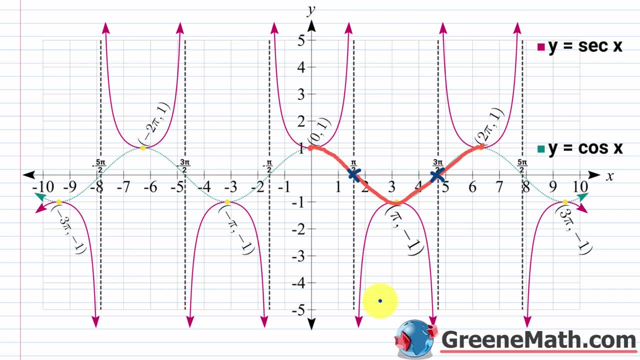 over two. Because, again, when you have the cosine function you're going to have a shared point: Cosine of pi over two, you get zero. we have the cosine of three: pi over two, you get zero. So those are x intercepts And therefore that's going to make your secant function undefined, because you 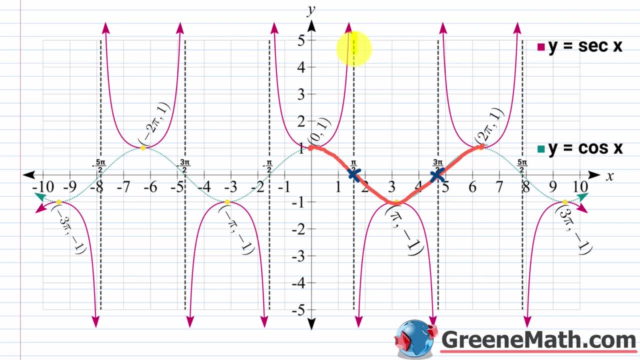 can't divide by zero, So you're going to get those vertical asymptotes at those values. So this is what you want to focus on here. Now that's going to change a little bit when we get to shifting the graph up or down, And I'll explain how to compensate for that. But right now we're just 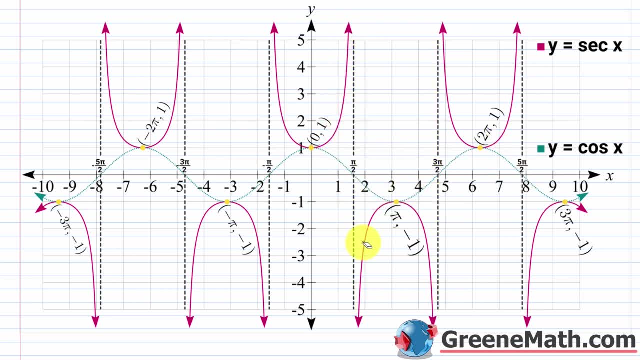 going to learn it this way. So when you think about this all together, just going over the whole graph that we have here, you would say that wherever the y value is one, you're going to have a shared point. So that's going to happen at an x value of zero, and then 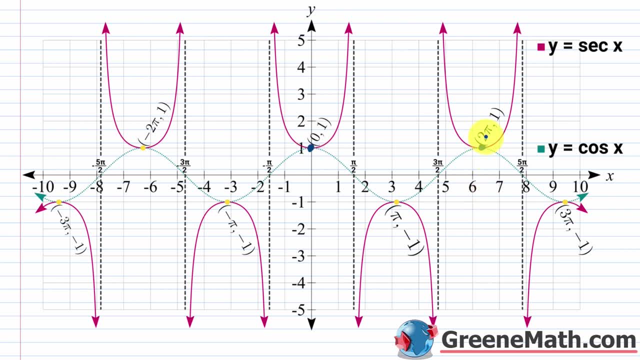 an x value of two pi, and then four pi, six pi, eight pi, so on and so forth. And then, going this way, you'd have negative two pi, negative four pi, negative six pi, so on and so forth. So you 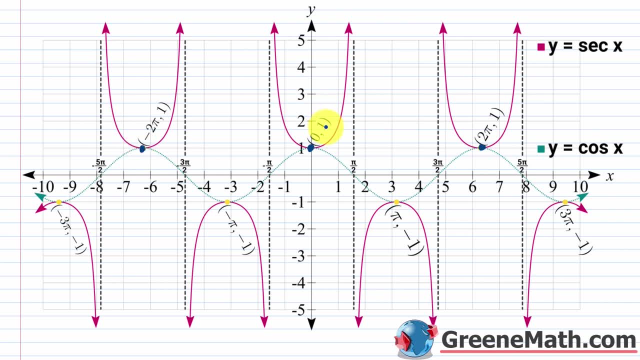 could say: at two pi? n, where n is an integer, the y value would be one and you're going to have a shared point between your secant graph and your cosine graph. Then, similarly, when you think about having a y value of negative, one, again that's going to have a shared point. So something like: 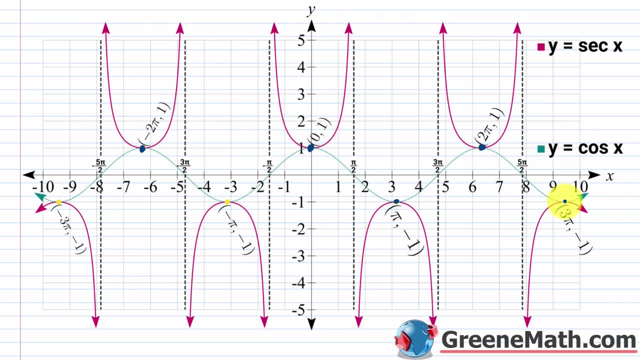 let's say pi comma negative one, And if you add two pi to that you'd have three pi comma negative one. If you subtracted away two pi from this pi here you'd have negative pi and then comma negative one. And then here's your negative three pi comma negative one. So 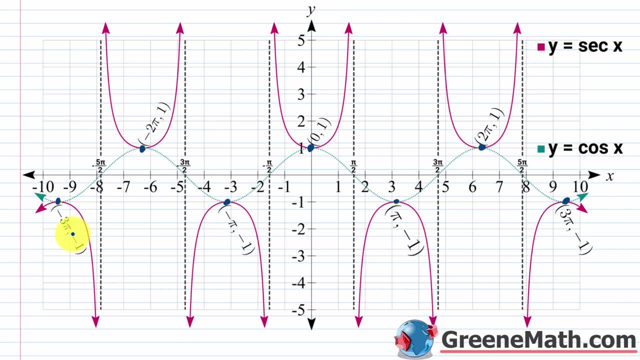 this would be at pi plus two pi n, where n is an integer. So five pi comma negative one would be there. seven pi comma negative one would be there, something like negative. five pi comma negative one would be there, so on and so forth. The idea here is: you want to think about that as being shared. 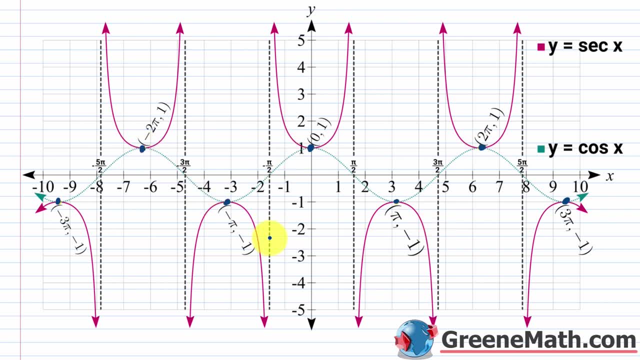 points, because when you see that there's a shared point, you're going to what we call interchange: the hills and the valleys. So what I mean by that is, when you think about the graph of cosine, you know that you have a maximum point anywhere where the y value is one and a minimum. 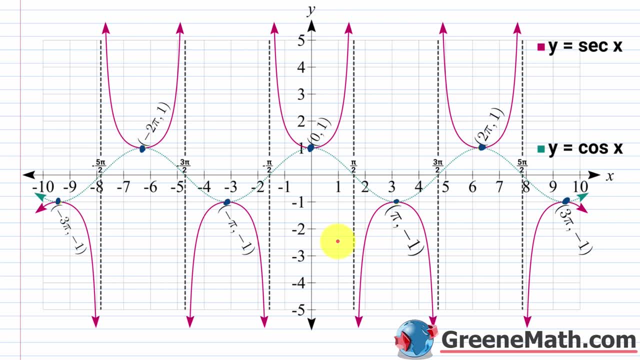 point anywhere where the y value is negative, one, because the range of cosine is from negative one to positive one, with both being included. So here you'd have a maximum point, and then again here, and then here. So when you think about it, this maximum point right here corresponds to what we. 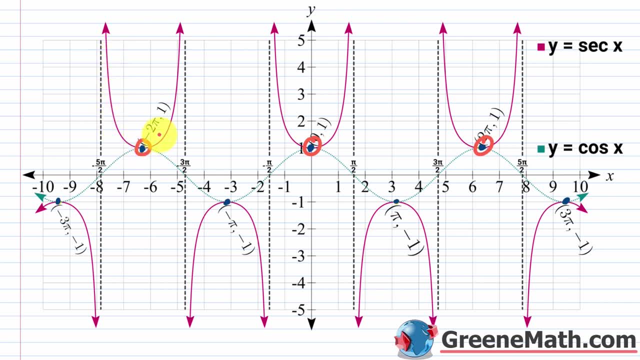 call a local minimum point on the graph of the secant function. So this right here is a hill and this right here is a valley. So the hills and the valleys are going to be interchanged. So this is a hill valley. Then, when we get down here, let me use a different color. you think about the fact? 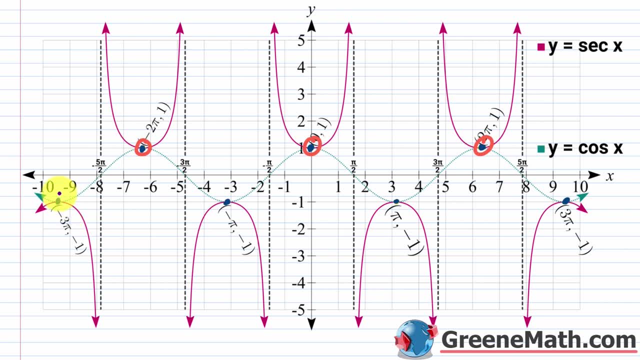 that okay. now when we look at our cosine graph, this is going to be a valley or a minimum, and then here this would be a local maximum or a hill, And then, when you come here, it's the same thing. So 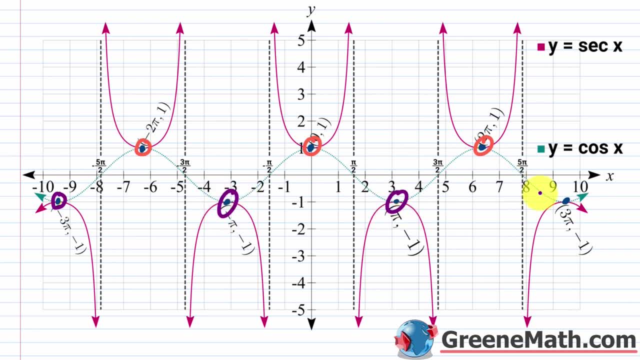 this is a valley, this is a hill Valley, and then this is a hill. You have a valley and then this is a hill. So that's all you really need to memorize. The hills and the valleys will be interchanged. 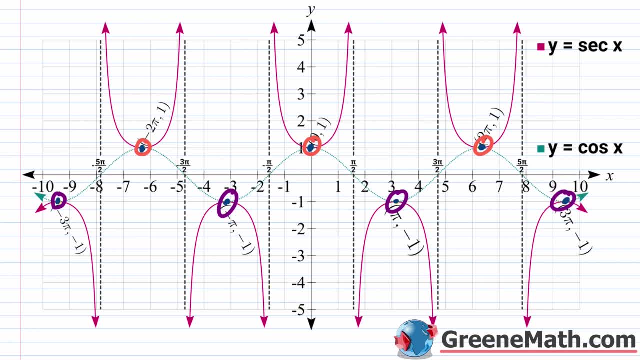 That's how pretty much every book says it and that's how I remember it. Now, the last thing again, like we talked about a moment ago, get these vertical asymptotes. So without shifting the graph up or down you're going to think about. 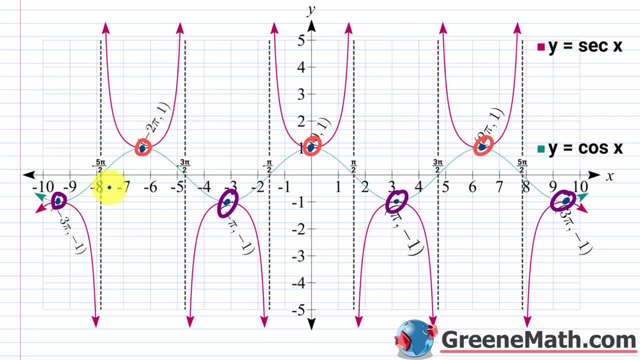 where are the x-intercepts for the guide function, the cosine function? Again, that's going to happen in odd multiples of pi over 2.. So at this: negative: 5 pi over 2, negative, 3 pi over 2, negative pi. 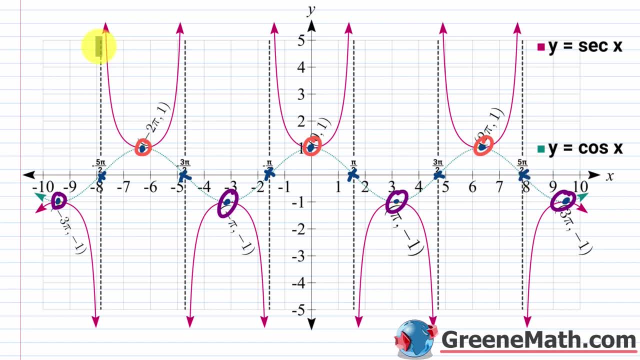 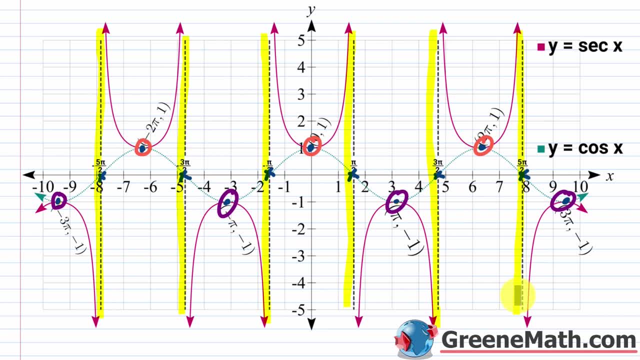 then here And again. this continues forever. So you would have 7 pi over 2,, 9 pi over 2, so on and so forth. All right, let's just go through the characteristics of the secant curve, So the 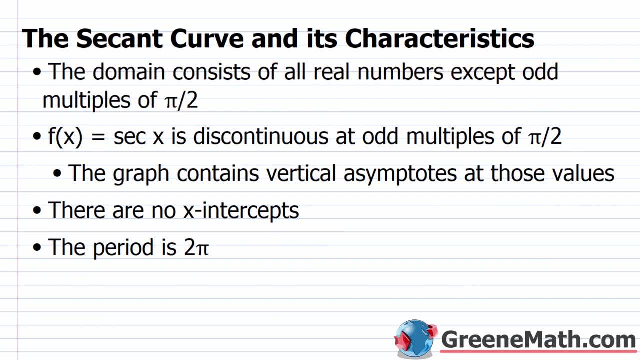 domain consists of all real numbers except odd multiples of pi over 2.. Again, this is because at odd multiples of pi over 2, you're going to get a cosine value of 0, division by 0 is undefined, So f of x equals the secant of x is discontinuous at odd multiples of pi over 2.. The graph contains: 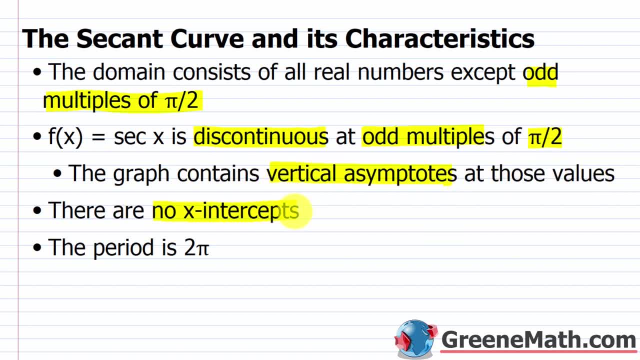 vertical asymptotes. at those values. There are no x-intercepts. You will only see those if you start shifting the graph up or down, And then the period is going to be 2 pi. So there are no minimum or negative values at those values. So you're going to get a cosine value of 0, and then the period is. 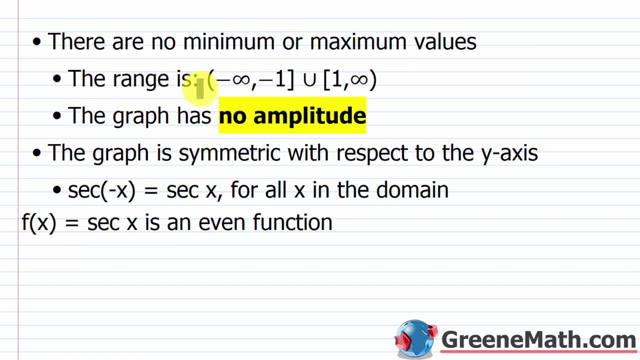 or maximum values. We saw that the range is from negative infinity going up to negative 1 and including negative 1, and then the union width you have from 1 and including 1 out to positive infinity. You will not see any y values between negative 1 and positive 1,, again because of the 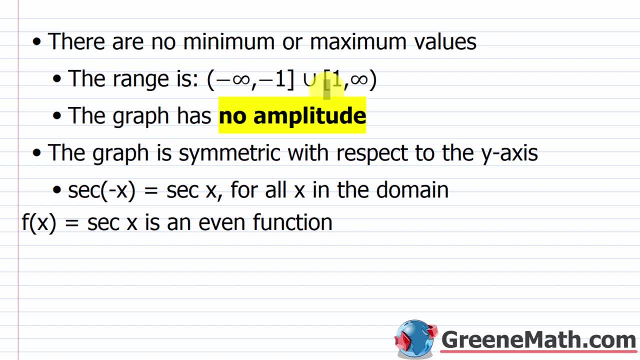 range of the cosine function, which is from negative 1 to positive 1, and the definition of the secant function, which is 1 over the cosine of x, Again something we talked about earlier when we were describing the behavior of the graph. So the graph has no amplitude again, because there 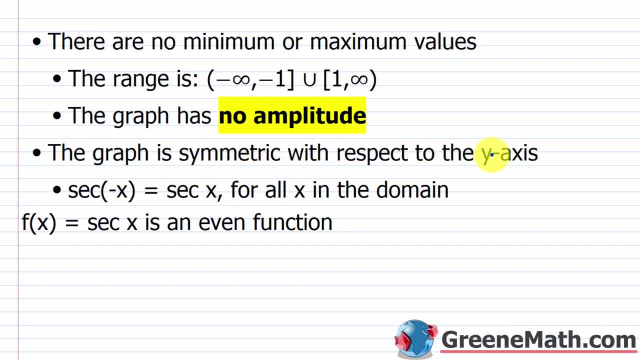 are no minimum or maximum values And the graph is symmetric with respect to the value of the y-axis. So the secant of negative x is equal to the secant of x for all x in the domain. So we can say f of x equals the secant of x. That is an even function, just like cosine. All right, so real. 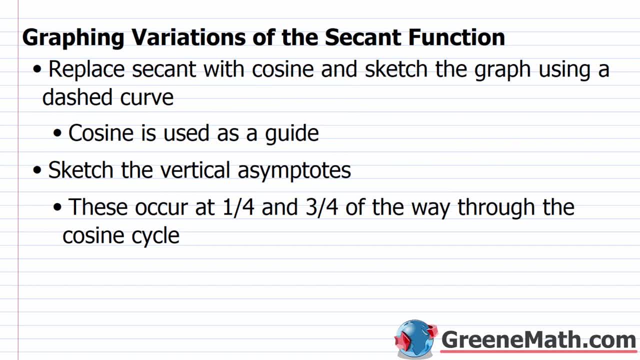 quick. we have a graphing procedure And you can write this down if you want. It's something you can just memorize if you don't want to write it down, It's not a big deal. So graphing variations of the secant function: The first thing you want to do is replace the secant with cosine and sketch. 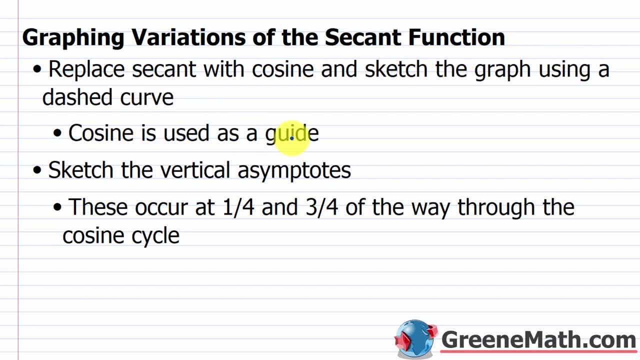 the graph using a dashed curve, So cosine is used as a guide. Then you want to sketch the vertical asymptotes, So this is the one that you're going to use to draw the graph. So you're going to really might have trouble with this step right here, And the reason for that is is that if you 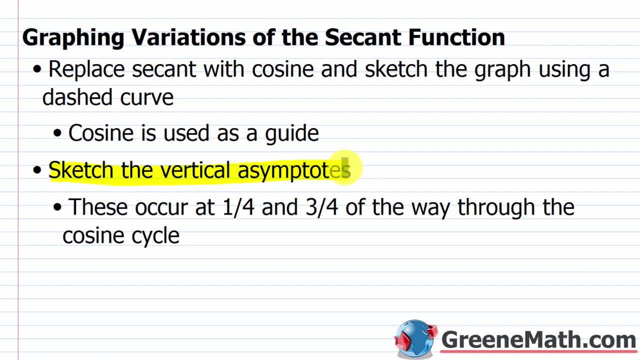 get a vertical shift involved, then you're not going to look for the x-intercepts of the cosine function or the guide function. It's going to be moved around And I'll show you that when we get to an example. The way I remember it is: these occur at a quarter of the way and three quarters. 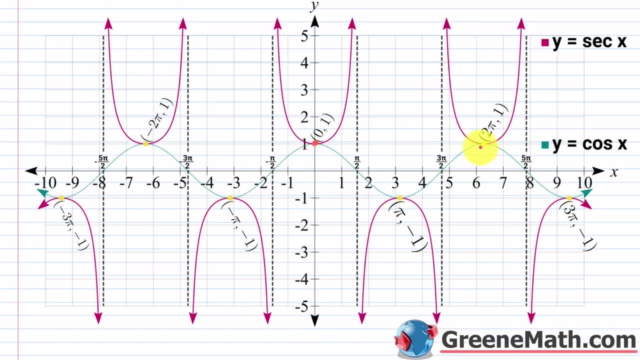 of the way through the cosine cycle. Again, just going back to this, here is the cosine graph, If you look at it over one cycle. So if we look at it over one cycle, it looks like that. So at the start of the cycle your x value is zero. So if you look at it over one cycle, it looks like. 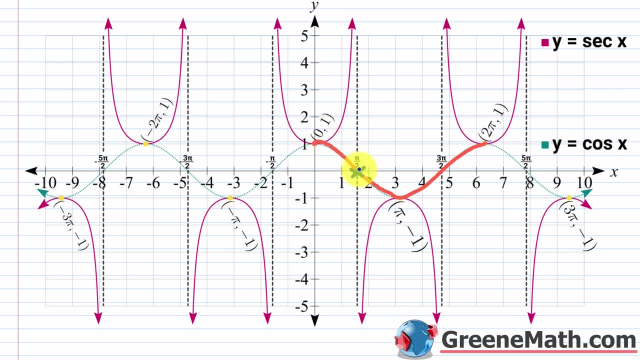 zero. When you get a quarter of the way through, your x value is pi over two, So you have an x intercept. When you get to the middle, your x value is pi three quarters of the way through, your x value is three pi over two. So you have an x intercept. and then you finish up at two pi for. 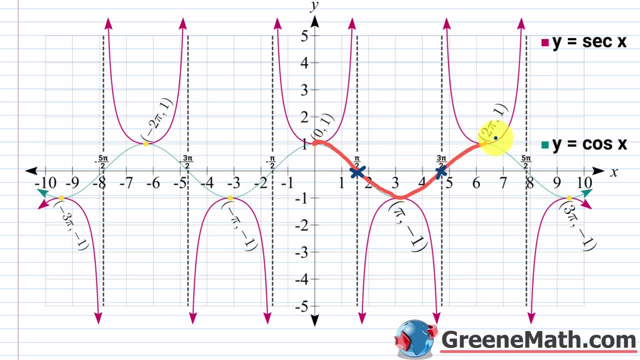 the x value. So zero pi over two pi, three pi over two and two pi. So just keep that in mind When we look at these variations of this guy. we're going to use the same thought process. So a quarter of the way through and three quarters of the way through. that's where we're going to have. 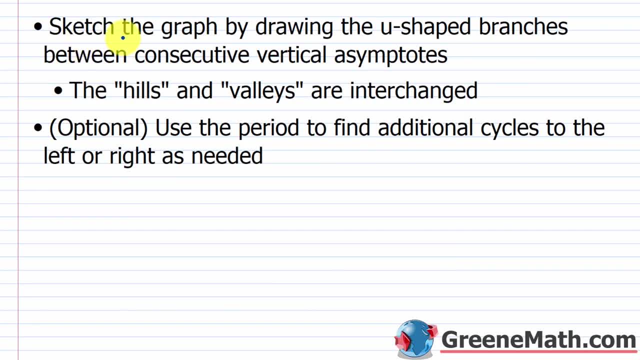 our vertical asymptotes for the secant function. All right, we have. sketch the graph by drawing the u-shaped branches between consecutive vertical asymptotes. So you have that the hills and the valleys are interchanged. So all you're going to do is you're. 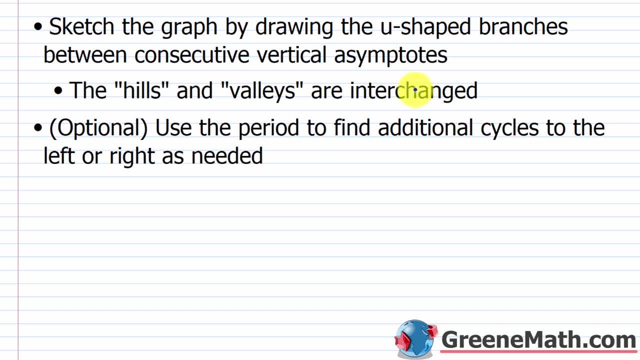 going to take those shared points. You're going to start there, You're going to make your u-shaped branches and you're going to approach your asymptotes but not touch them. Then we have optional here. Use the period to find additional cycles to the left or the right as needed, And 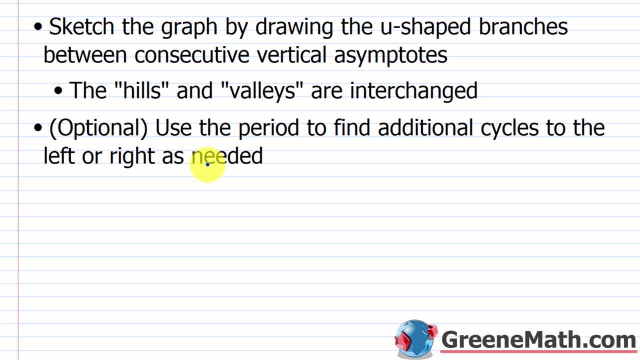 again, if you're self-studying, I would just do one period and call it a day. Usually, if you're given an assignment, your teacher will say: hey, I want you to sketch it from this place to this place, So just follow that. Okay, let's take a look at. 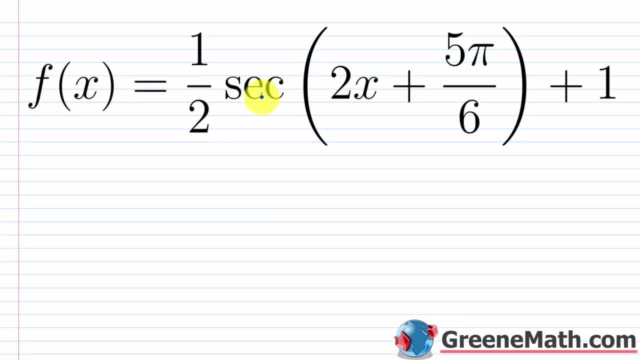 an example now. So we have f of x equals one half secant of two x plus five, pi over six and then plus one. So instead of just going straight into replacing secant with cosine, let's just get some information. So let's just go ahead and say that we have f of x is equal to one half, and then the 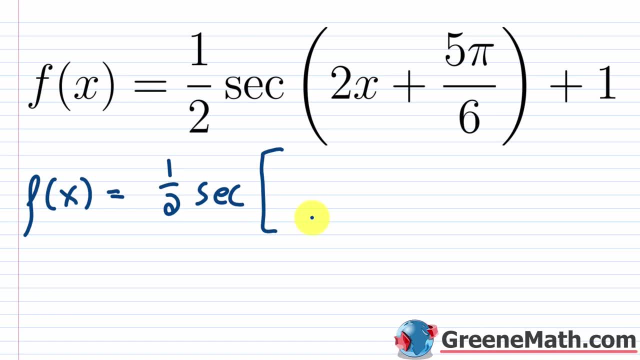 secant of. I'm going to factor out the two. Just makes it easier to find the phase shift. So pull that out. You're going to have x plus. how do I undo multiplication by two? I would divide by two or multiply by a half, So this would be five pi over six times a half, which is five pi over 12.. 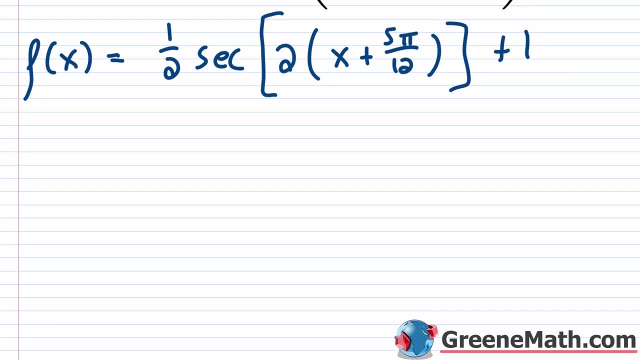 And so when we look at it now, finding the phase shift is very easy. You just want to say inside the parentheses here: how do I undo what's being done to x? We have this plus five pi over 12. To undo that you want to subtract away five pi over 12.. So for the phase shift you could say minus. 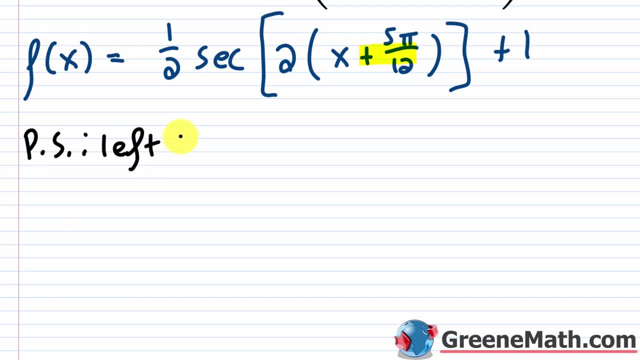 five pi over 12, or most people will just say left five pi over 12.. Now, in terms of the vertical shift, it's very straightforward. So you have this plus one here. So the vertical shift, that's just going to be up one. Now thinking about the period, so we'll need that. So what is the period? 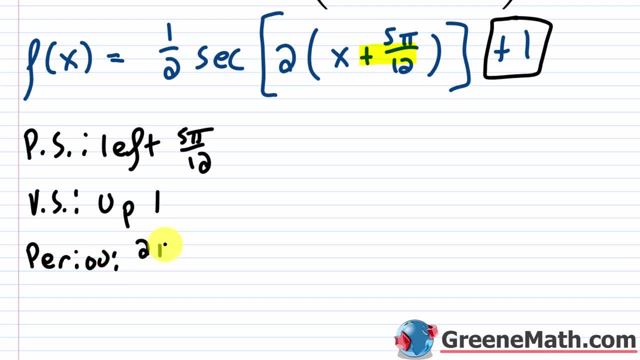 for this guy. Again, the standard period is two pi when you're looking at either sine cosine secant or cosecant, And we're just going to divide that by the number outside the parentheses here, If it's an unfactored form, it's the coefficient of x. So two pi over two, which would 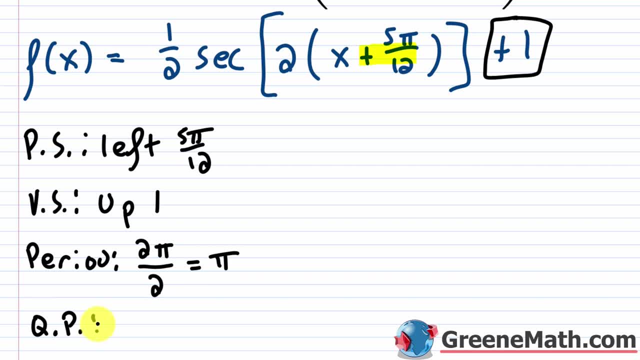 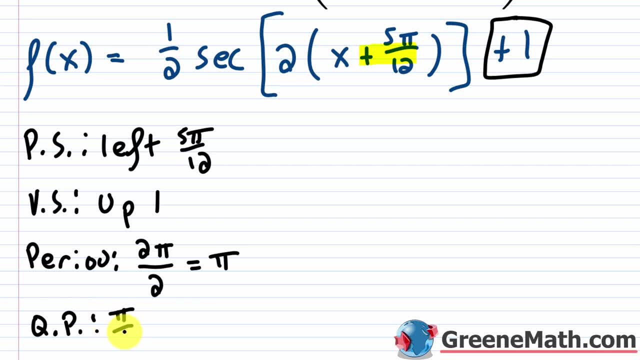 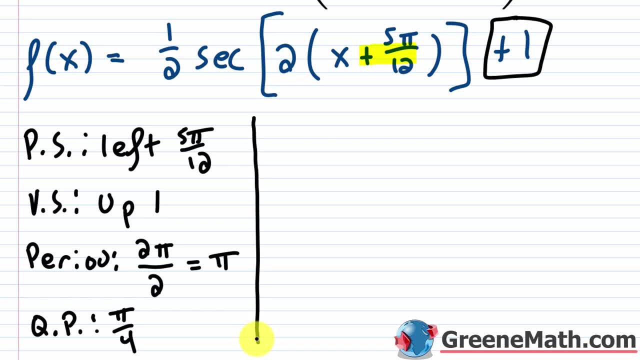 I'm going to talk about the graphing transformations, And you can use this method if you want, or you can use a different method. is really going to be up to you. So, in terms of x, remember, this is the one that's really hard for students. That's why a lot of people just turn to the quarter. 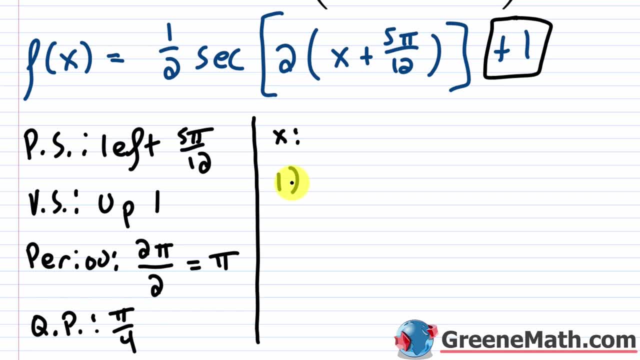 period method, Because this becomes a little bit challenging to remember. you need to undo what's being done- x- And so to undo something, you have to go on the reverse order. Think about writing a document or something like that. you hit Ctrl Z, you're undoing the latest thing you did. you don't. 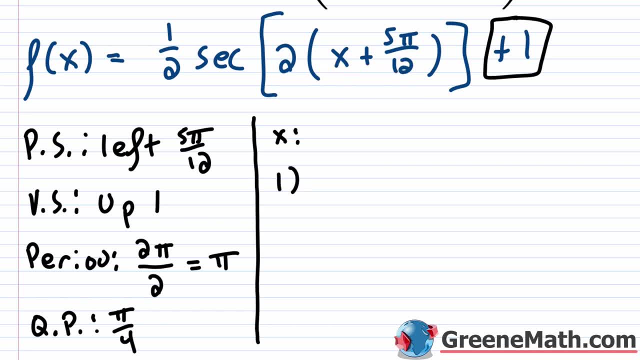 undo the first thing you did. So if you look at the order of operations here again you have parentheses here And I know you could distribute that to n, but we're not doing that here. So from the order of operations we know we would work inside the parentheses first and then do the 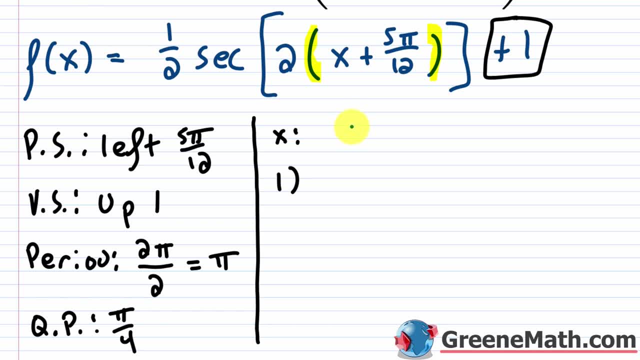 multiplication second. So if I write this out now, I have to go in the reverse order. So this would be one and this would be two, and each thing has to be undone. So how do I undo multiplication by two? I would divide by two or multiply by half, So you would multiply. 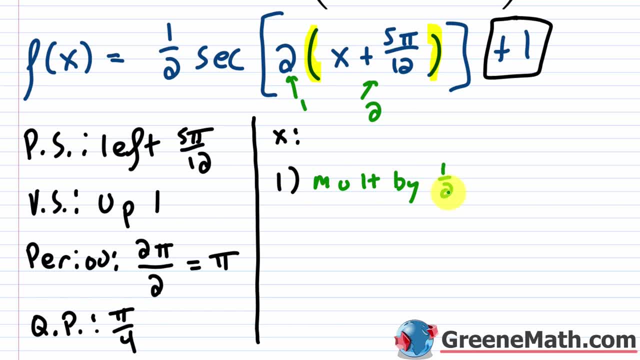 by one half. So that's giving me a horizontal shrink by a factor of a half. I know a lot of teachers will also say this as a horizontal compression by a factor of two. Again, I don't want to get caught up on the terminology. A lot of people get confused by those two ways of saying. 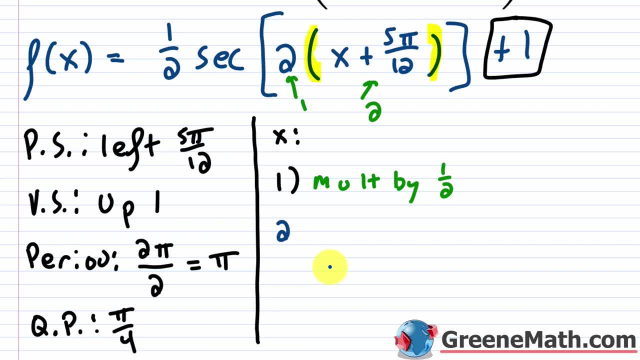 the same thing. Just realize that you're having your x coordinate either divided by two or multiplied by half. Then the second thing is: you want to undo this plus five pi over 12.. Well, we want to subtract five pi over 12.. Again, we saw that earlier when we did the phase shift, that's: 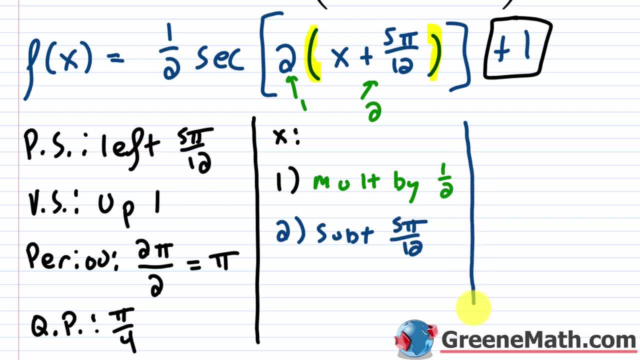 going to shift me to the left. five pi over 12.. Then, when you think about the transformations for y- these are the ones that are very straightforward- You have this one half here. that's multiplying this guy. So the first thing is you would just follow that. So multiply by one half. 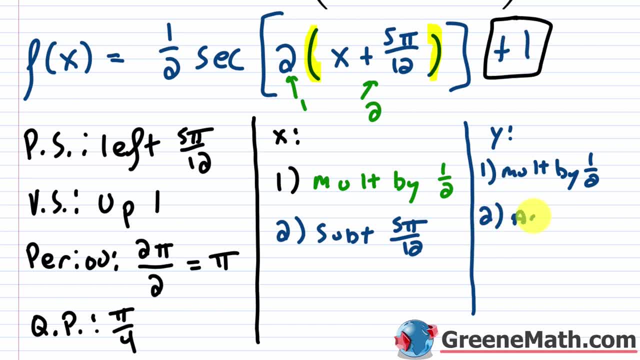 And the second thing is: you're adding one, So you're going to add one Again. this is straightforward. It follows the order of operations: You multiply before you add. So with this one you could say vertical shrink by a factor of a half, or you could say vertical compression by a. 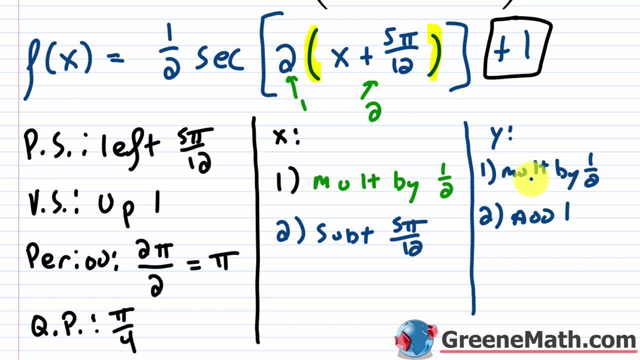 half. Again, I know that confuses people when you have two different ways to say the same thing. but just realize: you're taking the y coordinate and you're either dividing it by two or you're multiplying it by a half And then you're going to add one. that's shifting me up by one unit. 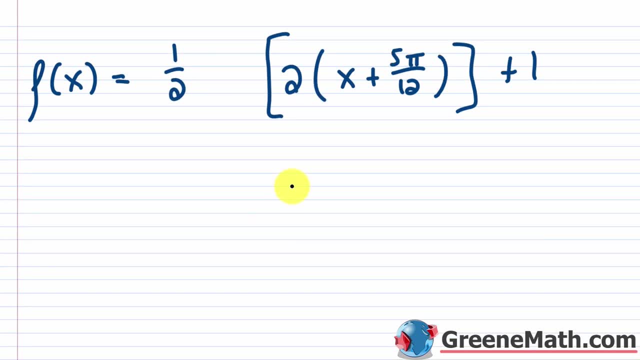 Okay. so, coming to a new sheet, here, I'm going to erase the secant and just put in cosine. So remember, we're going to graph this as a guide. So how do you graph this cosine function? Again, lots of ways to do it. You can use all graphing transformations. You can use no graphing. 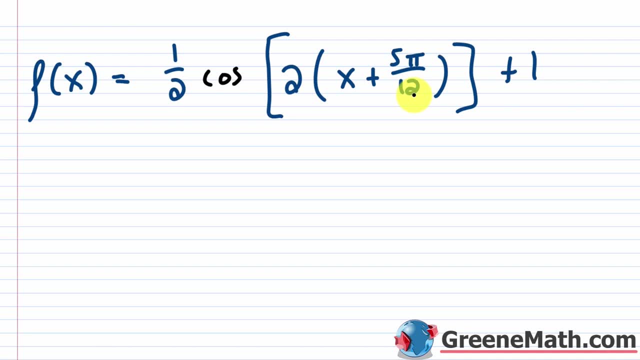 transformations. It's really up to you. So I'm going to do both the quarter period method and all graphing transformations method, And then on the next ones I'll just use the quarter period method because it's a little bit easier for students to understand. So when we think about 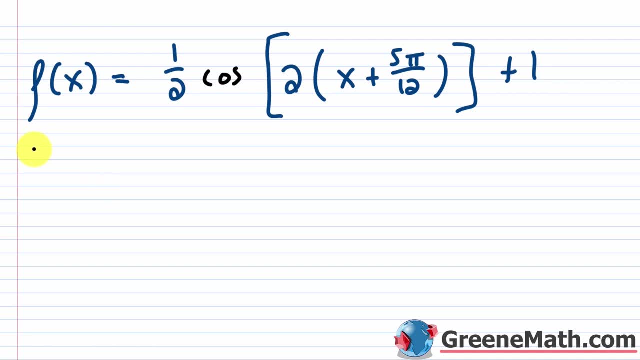 using the quarter period method. you start off by thinking about your points for the basic cosine function. So y equals cosine of x. you have a point, you start off at the maximum, so zero comma one, and then you're going to go to your x intercept. So this is pi over two comma. 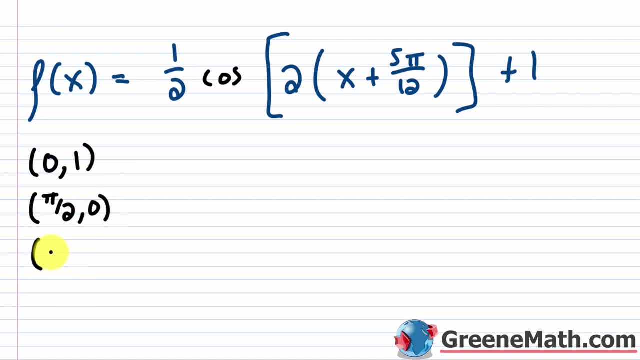 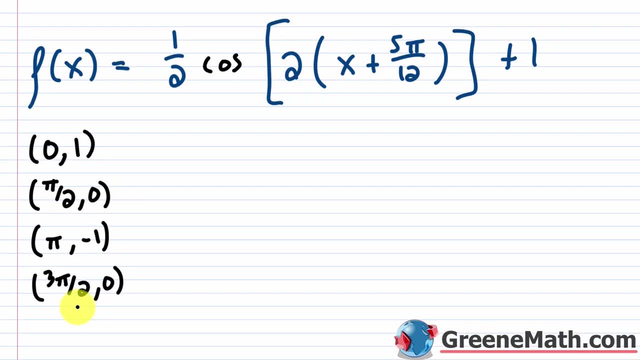 zero and then you're going to go to your minimum. So this would be at pi comma negative one. back to an x intercept. So this is three pi over two comma zero and then you're going to finish up at the maximum. So two pi comma one. So these are points you should have memorized at this point. 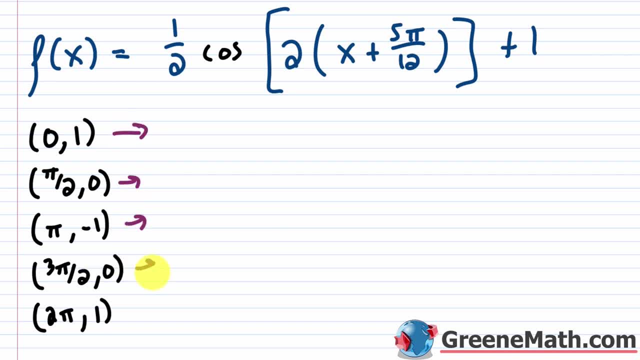 And all we're going to do is think about, for the first x value, here you just use the phase shift. In other words, you have this zero right here and I'm going to think about what is the phase shift? So we know it's to the left by five pi over 12, or you could say I'm subtracting away. 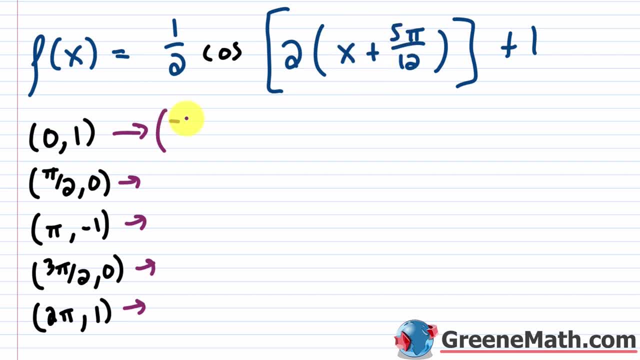 five pi over 12.. Again, I've got to undo what's being done to x there. So this x coordinate would be negative five pi over 12 right there. To get the additional x coordinates here, all you're going to do is you're going to take this value right here, Don't worry. 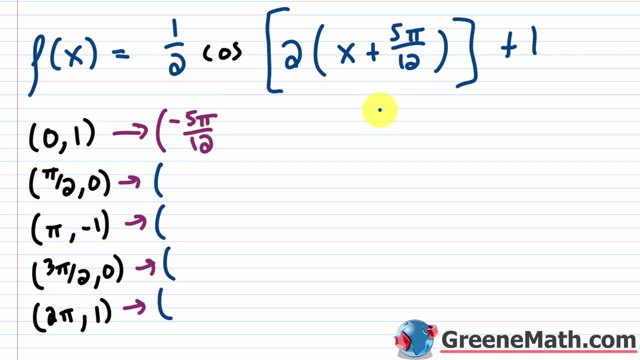 about these, This value right here, and you're going to keep adding quarter periods. So the quarter period again was pi over four. You took your period, which is pi divided by four. Here I'm going to multiply this by three over three. So we have a common denominator. So it's three pi over. 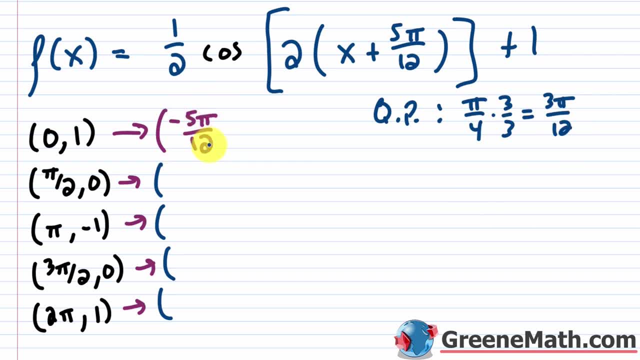 12.. So you're going to keep adding three pi over 12.. Again, start here. negative five pi over 12 plus three pi over 12. That would give me negative two pi over 12.. I know you could simplify that, but let's just hold off for a moment. So we have a common. 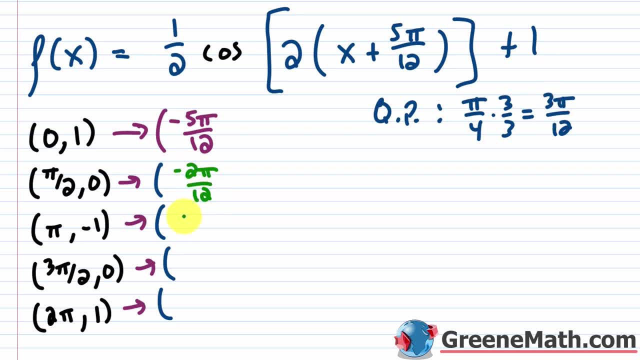 denominator So negative. two pi over 12 plus three pi over 12. That would give me pi over 12.. Then pi over 12 plus three pi over 12. That's four pi over 12.. Again, don't simplify it yet: Four pi over 12. 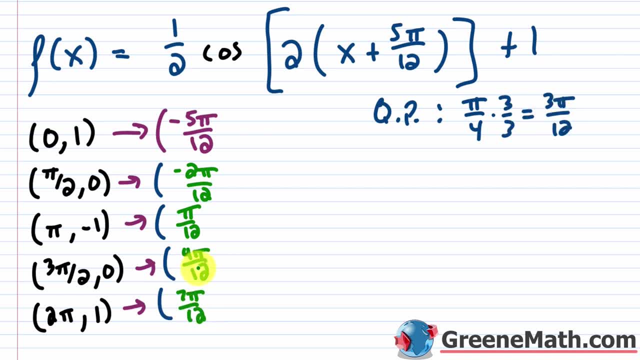 plus three pi over 12.. That's seven pi over 12.. Now this right here, this four pi over 12, you could write that as pi over three. So this is pi over three And then negative two pi over 12,. 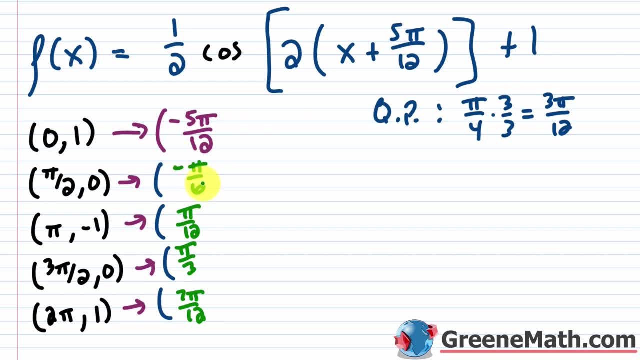 you could write that as negative pi over six, So negative pi over six. Let me make this better here. Go on. I want to show you that you can get the same values here just using those graphing transformations that we talked about a moment ago. So, coming back up here, let me grab this. 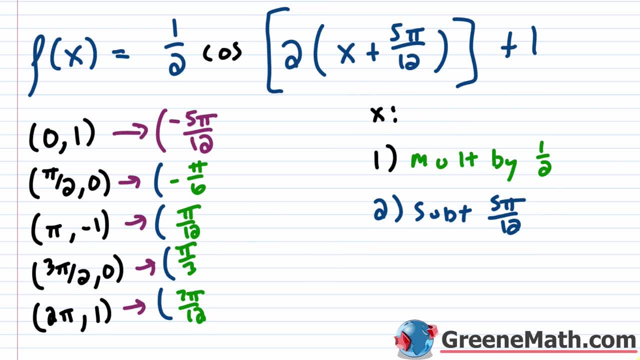 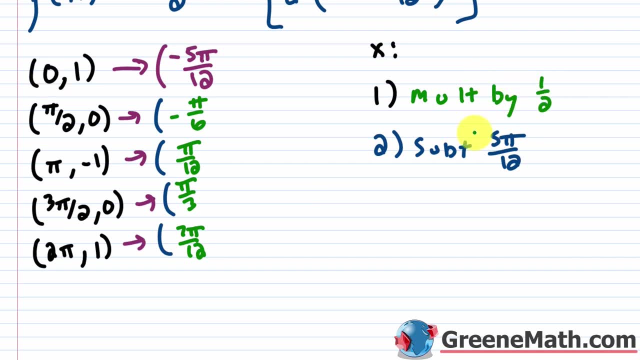 real quick and come down here and paste this in, And I'll just do the first two of them, because this is a little bit time consuming. So for this one, you stick with these guys right here. So for zero, you multiply by half. you get zero. Then you subtract five, pi over 12, you'd have negative five. 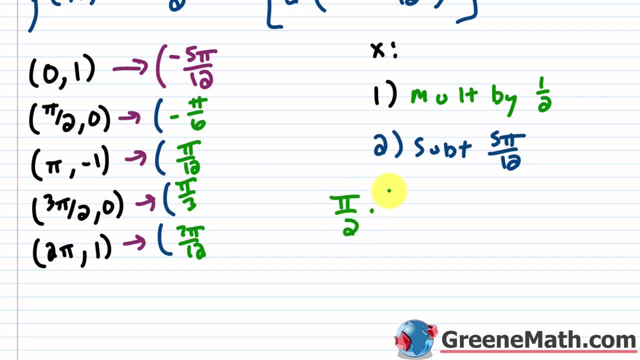 pi over 12.. Then you would take pi over two and multiply by a half. So you do that first And then you're going to subtract away five pi over 12.. So this is very tedious because you have to get these common denominators. So this becomes pi over four minus five pi over 12.. So we'll say this: 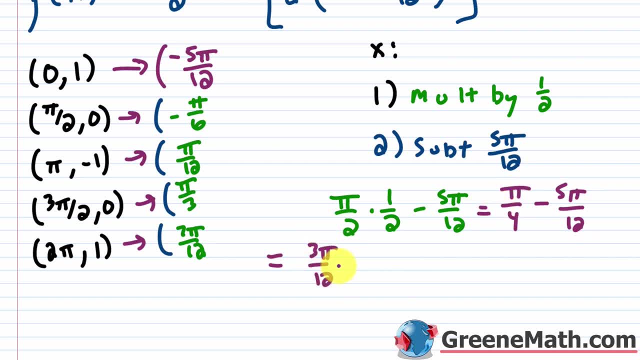 is: let's multiply this by three over three, So three pi over 12, minus five pi over 12,, which becomes negative two pi over 12, which is going to simplify to negative pi over six. So you see, you have negative pi over six there. Let's just do one more. I don't think we have to do all of. 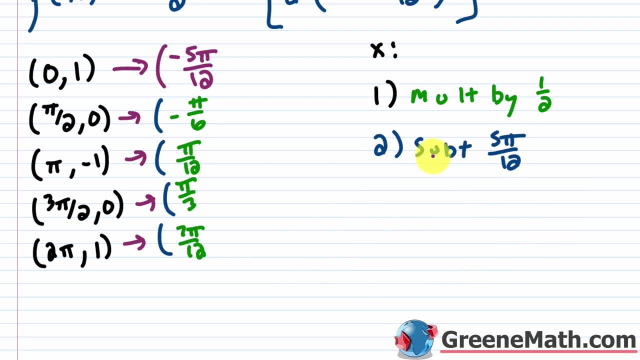 them. You can do them all on your own. This is just to show you that you have different techniques to use. So we have multiply by a half. So let's start with pi And we multiply by a half And five pi over 12. So this becomes pi over two minus five, pi over 12.. Multiply this by six over. 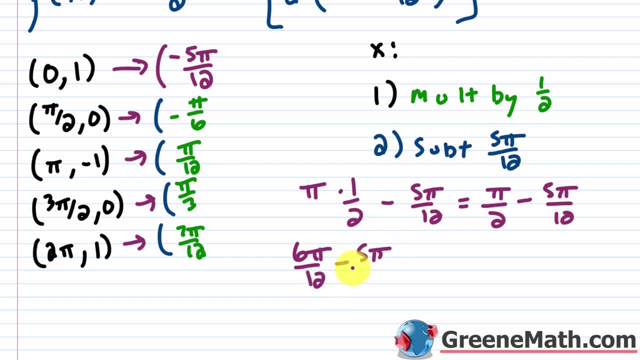 six. So you have six pi over 12 minus five pi over 12.. So this would give you pi over 12.. So pi over 12 there. So again, if you follow this, you'll get the same result as using the quarter. 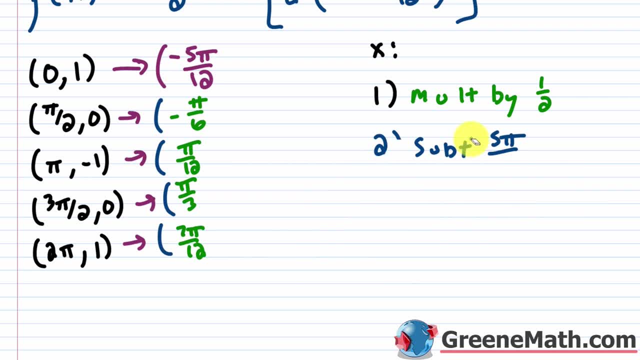 period method. I know a lot of students do not like using graphing transformations for x because the procedure itself is hard to get And then in this case it would be a little bit more tedious than what we did with adding quarter periods. So we have our x coordinates. So that's the first. 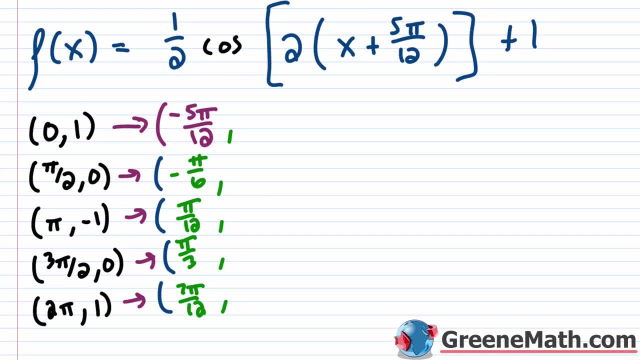 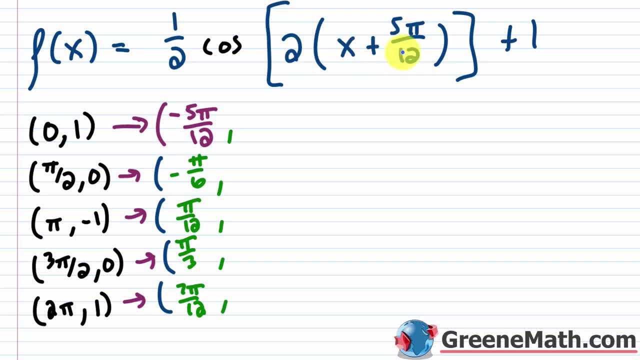 negative. five pi over 12 plus five pi over 12, well, that's going to be zero. Two times zero is zero, So you would get the cosine of zero, which is one. So notice that this right here when I go. 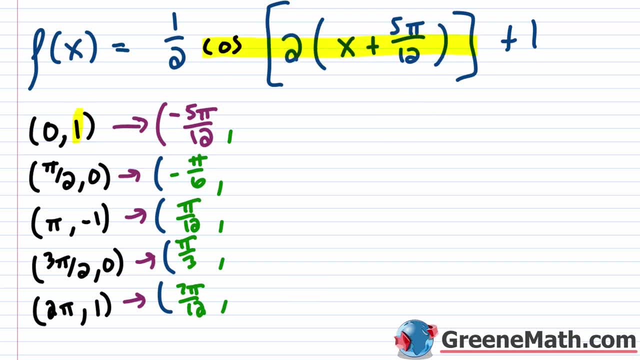 through the process, I get this y coordinate right there, So I could have shortcutted that and not plugged in and just said, okay, well, it's going to be one half Times, whatever this y value is, which is one, and then plus one Again if we go back. 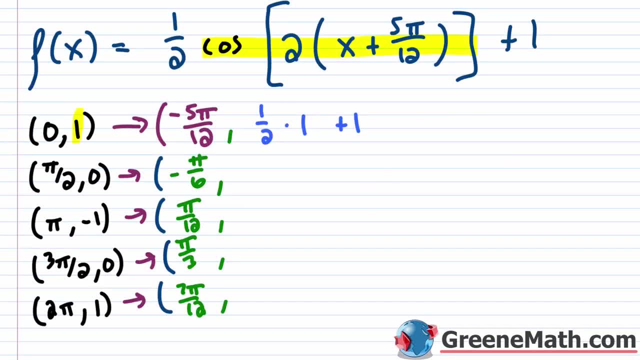 that's what we came up with here. Multiply by half and then add one. That's all you're doing. When you look at this one here again, if you plugged in- and I'll just do it for this one negative pi over six. if you plug that in there and you go through the steps, you're going to end. 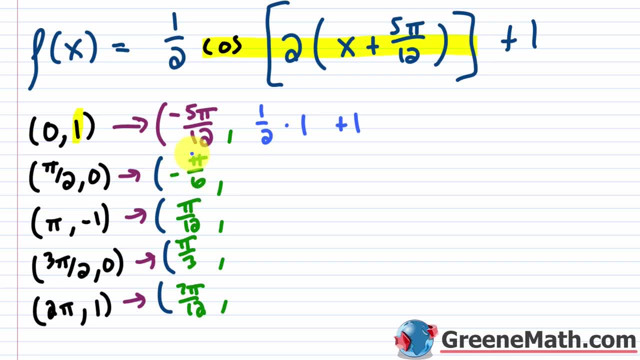 up with this guy right here being zero. Because when you plug in a negative pi over six and you go through the steps, you're going to end up with the cosine of pi over two. And let me just show you that real quick, just so that's crystal clear. If you did the cosine of, you have two times. 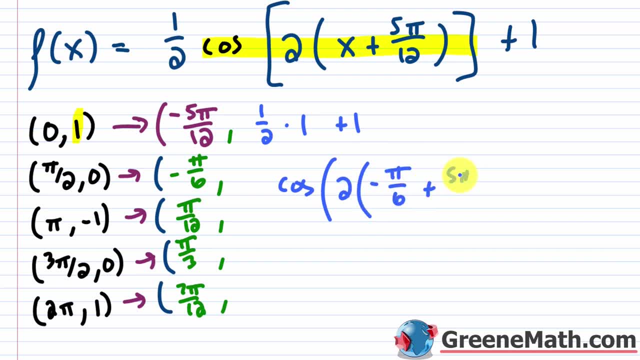 plug in negative pi over six and then plus five pi over 12.. Okay, so we just need this part right here. I'm going to multiply this by two over two, So this would be negative two pi over 12.. And what would that give me? Well, negative two pi over 12 plus five pi over 12, that's three pi. 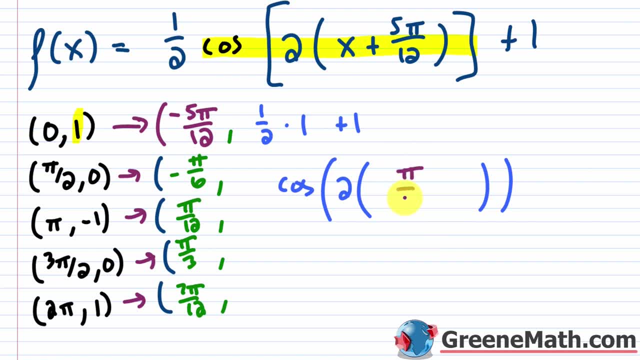 over 12.. And three pi over 12,, you can say, is pi over four. Well, two times pi over four, that's going to be pi over two. So the inside part here, this part right here, is going to be pi over. 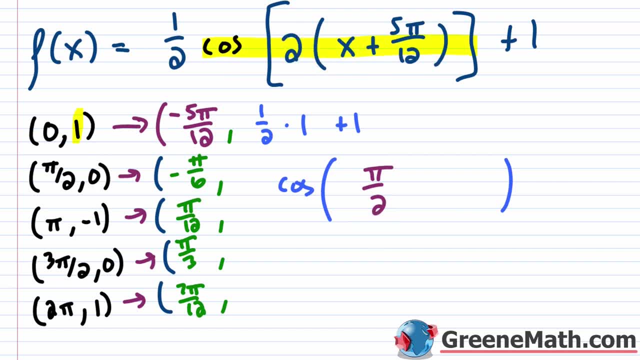 two, and the cosine of pi over two is zero. Well, notice, that's going to be pi over two again. the y coordinate there is zero. So all I had to do was sit there and say that I know that the result of this will be zero. So I can just say: well, it's going to be one half times zero. 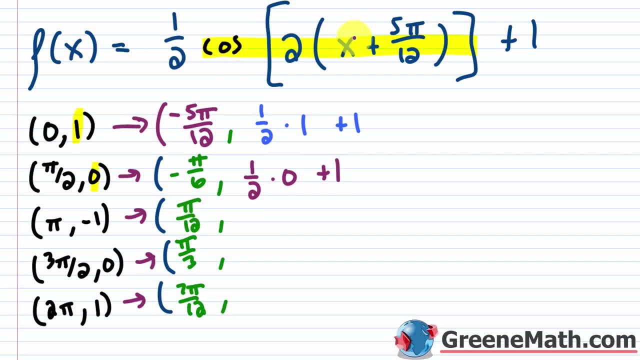 plus one, And then if I was to plug in pi over 12, the result of this part right here would be negative one. So one half times negative one plus one again, so on and so forth. These are just duplicates, so you don't have to do this. So I'm just going to say that this is one half times one. 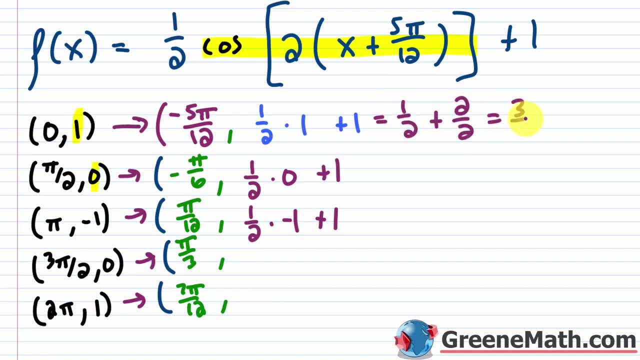 versus one half. plus let's write: one is two over two, So this is three halves. Then this one: anything times zero is zero, So this is just one, And then negative one times a half is negative one half, And then plus this will be two over two. 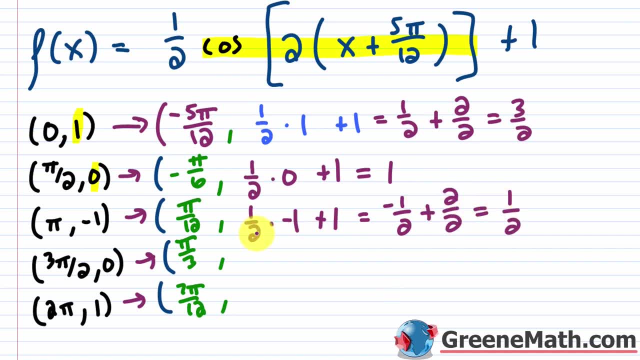 So this is one half. So this would be three halves, one and one half. Let me erase this and write those in. So this is three halves, one and one half, And again, for this one, it's going to be one again, And then, for this one, it's going to be three halves again. 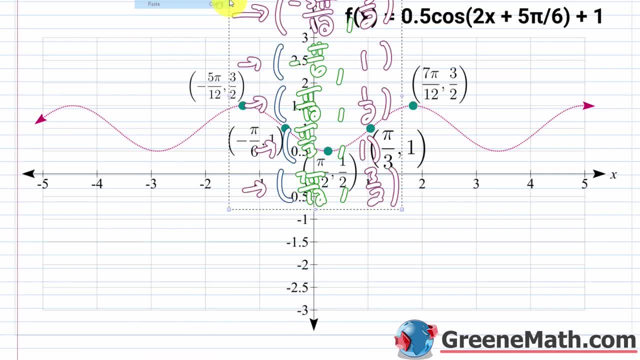 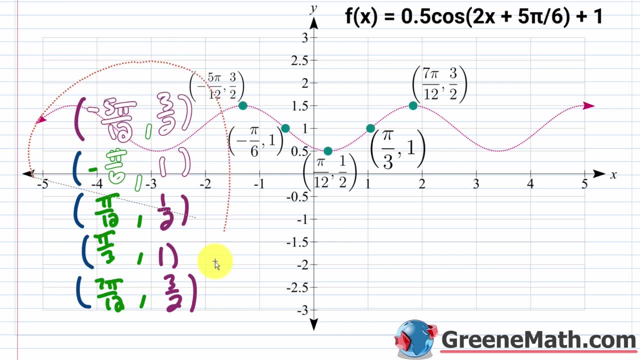 When we think about graphing this guy. let me grab this real quick. I have given you a link for all of these guys that we're going to look at today on Desmos, So just click on that if you want something that has a little bit of a difference between the two, So I'm going to 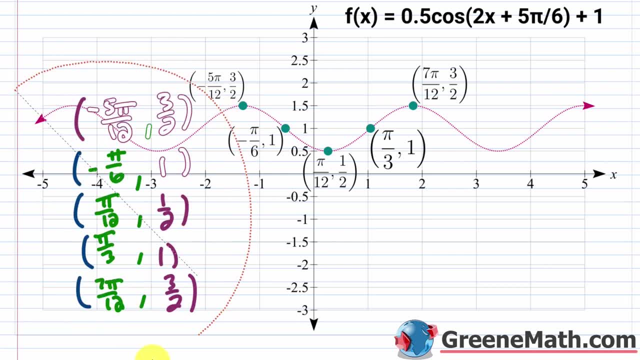 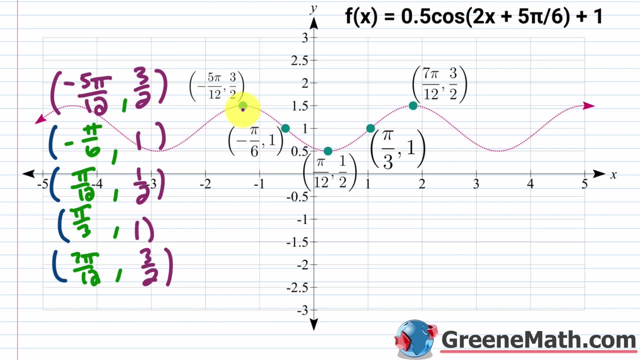 more detail or is easier for you to follow along with, So you can just pause the video and check these points out. When you see that this point right here again at the beginning of the cycle, you have negative five pi over 12 comma three halves, Then this right here is a quarter of the. 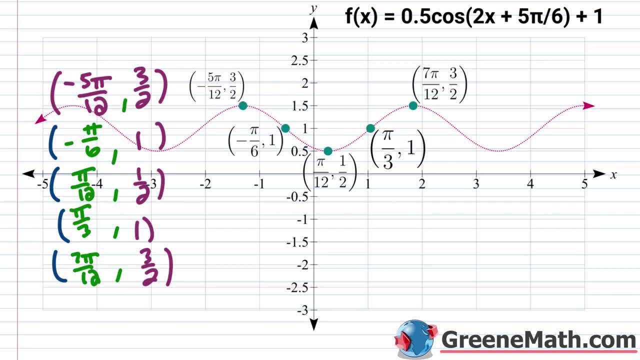 way through. You have negative pi over six comma one. So you want to focus on this one right here, because this X value is where you're going to have your vertical asymptote. It's always going to be a quarter of the way through And then you're going to have midway. you have pi over 12 comma. 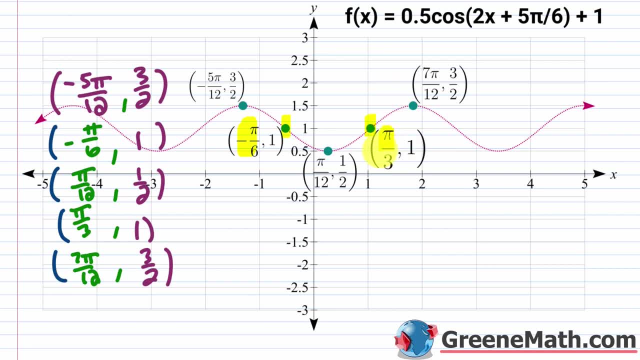 one half, And then this one right here is three quarters of the way through. Again, that's where you're going to have a vertical asymptote. there You're three quarters of the way through. So pi over three comma one. And then you're going to the end of the cycle. So seven pi over 12 comma. 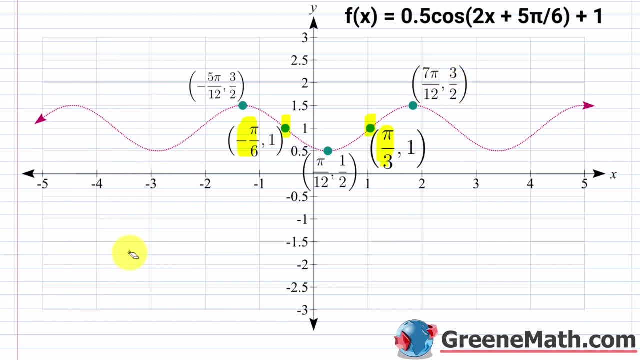 three halves. What a lot of teachers will do is they will draw a horizontal line which in this case would be: y equals one. They're showing you that the midline of this guy has been shifted up by one unit. So this right here would be: y is equal to one. So a lot of students will do that. 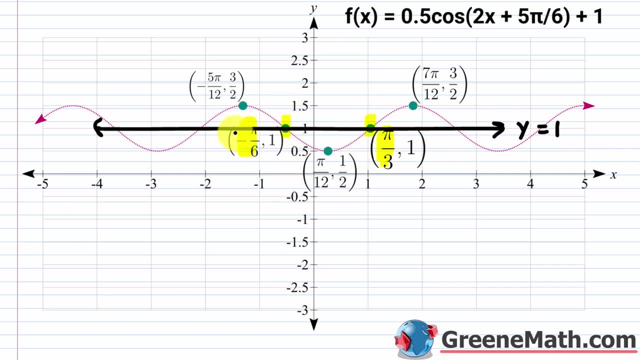 instead of remembering that it's at the quarter and three quarters and just say, OK, well, anywhere in the line, well, this has been shifted up like that, So I'll look at the X coordinate. In this case, it's negative pi over six. It's covered up a little bit. In this case, it's pi over three. 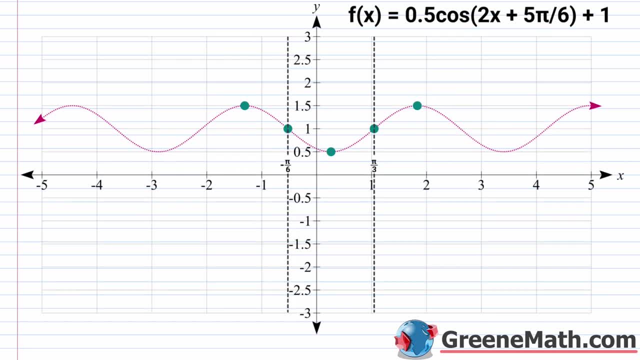 And that's where I'm going to have the vertical asymptotes drawn. So go to the next graph. That's what we have. So here's your X equals negative pi over six. Here's your X equals pi over three. That's all you're focused on. This is a quarter of the way through and three quarters of the way. 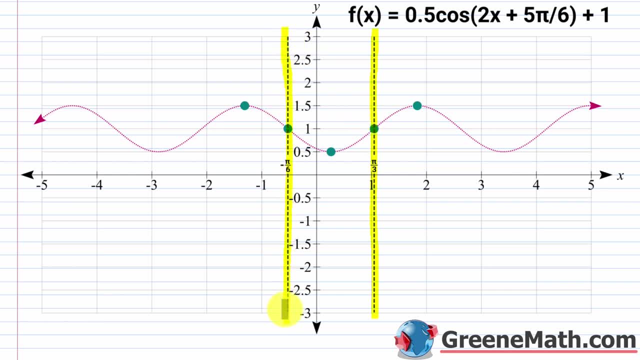 through. That's how you want to draw this in terms of getting the vertical asymptotes for the secant function. Now, once you have that, you're ready to put everything together. So let me just highlight this again. So we have this vertical asymptote. 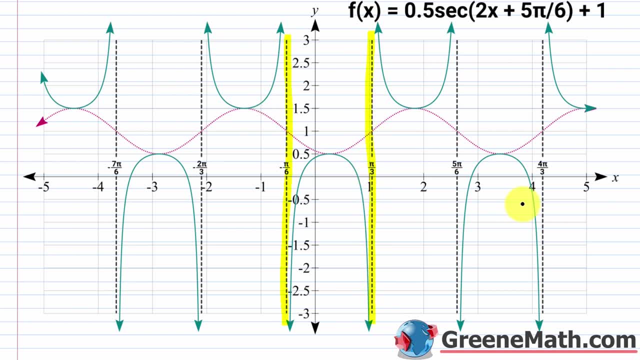 And this vertical asymptote. So this is extended to the left and to the right a little bit. But again, if you're doing this on your own, you're going to have this point right here, that we found, this point right here, that we found, and this point right here that we found, Again, this point right. 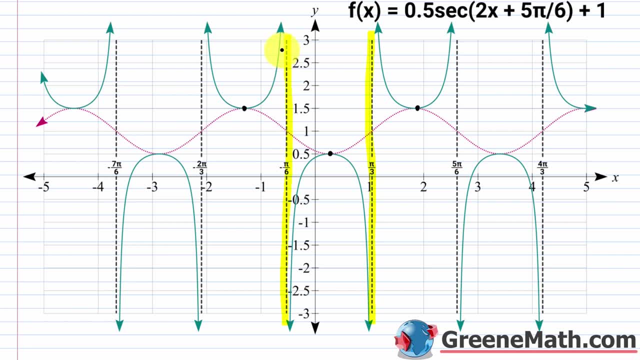 here. at this point, right here, that's not really relevant anymore because we use it to make the vertical asymptotes, So we don't need that. The idea is that, again, when you see a hill here, it becomes a valley here, So that means that this right here would be drawn to where it approaches. 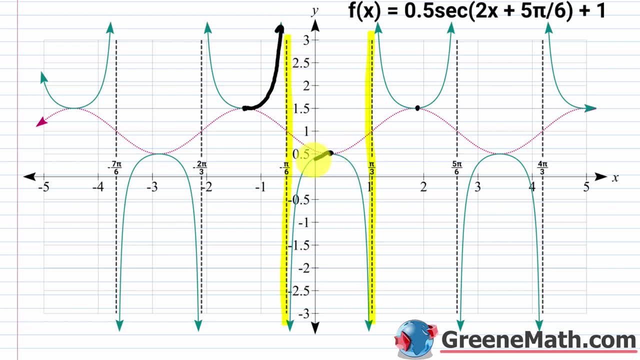 that vertical asymptote, And then this right here would be drawn to where it approaches the vertical asymptote. Same thing for this part, right here And again. the way you know that this is going down like that, this right here is going to be a. 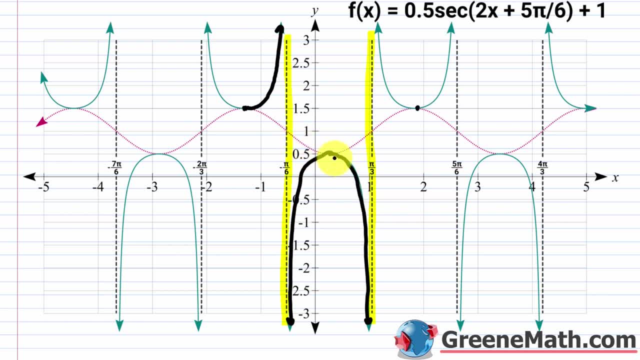 valley. So this right here becomes a hill. This minimum here becomes a local maximum here. This maximum here on the cosine guide is going to become a local minimum here. Then, when we look at this part right here, So again this is a hill, So this would be a valley. So this maximum here on 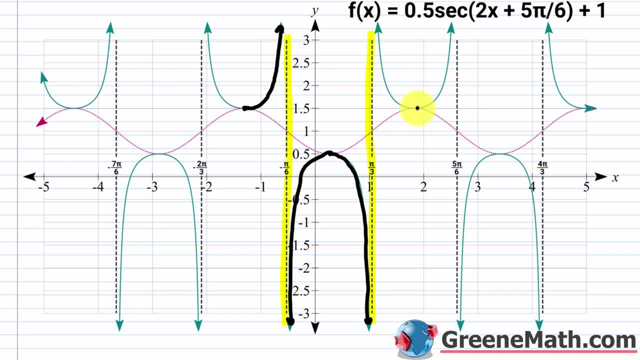 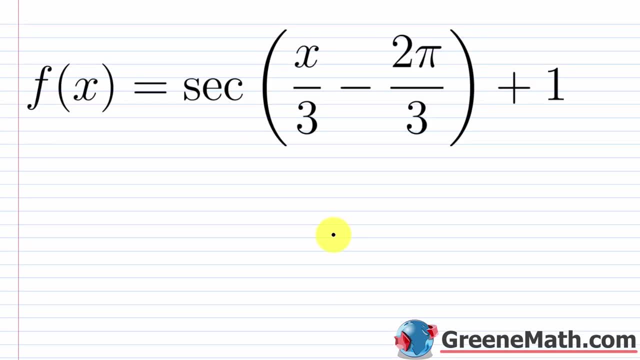 the cosine guide is going to be a local minimum on the secant graph. So this guy right here would be drawn to where it approaches the vertical asymptote and doesn't touch it. All right, let's take a look at another example with secant. So here we have: f of x equals the secant of x over three minus two, pi over three. 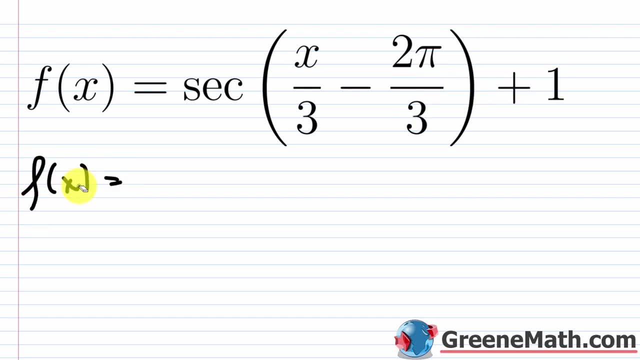 plus one. So again, let me just factor this guy so we can get the phase shift more easily. Let me make that a little bit better. So this is the secant of. I'm going to pull out a one third And this one's very straightforward. Let me slide this down so I have room. 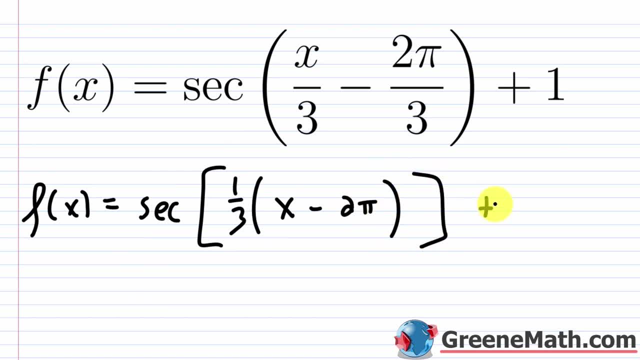 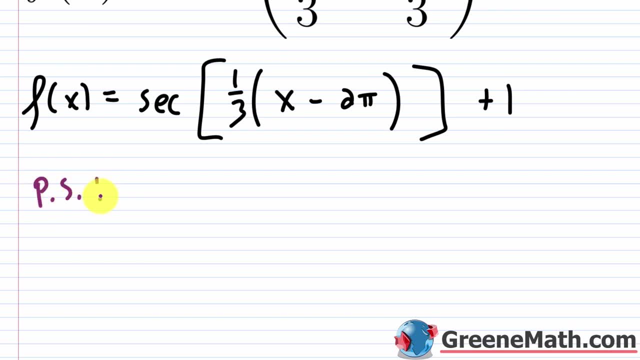 So we have x minus two pi. close that down, close this down, then plus one. Okay, so looking at this, just getting some information. If you want the phase shift which we're going to use with a quarter period method, you have to undo what's being done. x. so you have this minus two pi here. So I'm going 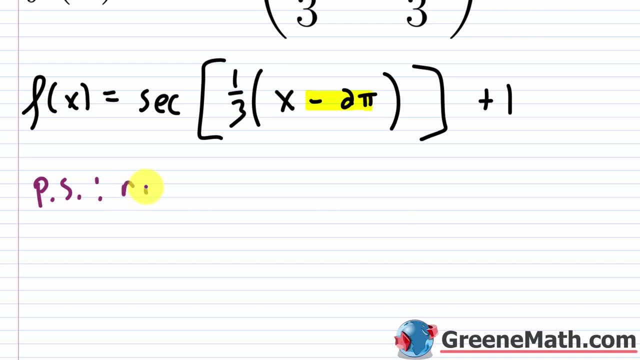 to add two pi to undo that. So that means I'm going to the right. So I'm going to the right by two pi. Then for the vertical shift, again you have this plus one here. So that means I'm going up one for the. 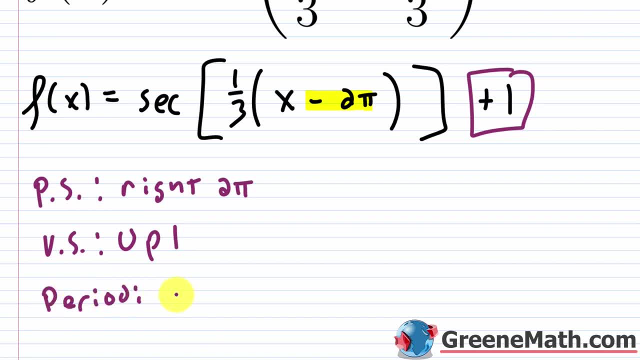 period. Again, you're going to take the standard period, which is two pi, And you're going to divide by this number, outside the parentheses, in factored form or if it's not in factored form, you had that x over three. So the coefficient of x is one third. So it's just two pi divided by a third, which is two. 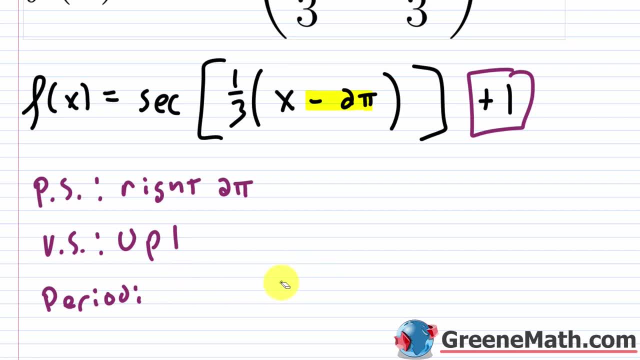 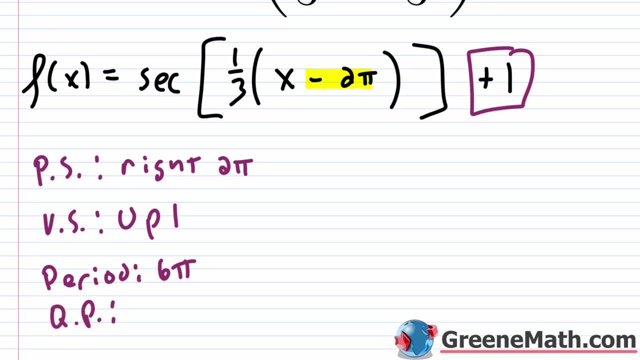 pi times three, which is six pi. So your period here is going to be six pi, And then the quarter period that's going to be six pi over four. Let me slide down a little bit. So six pi over four. six divided by two is three, And then four divided by two is two, And then six divided by two is three. 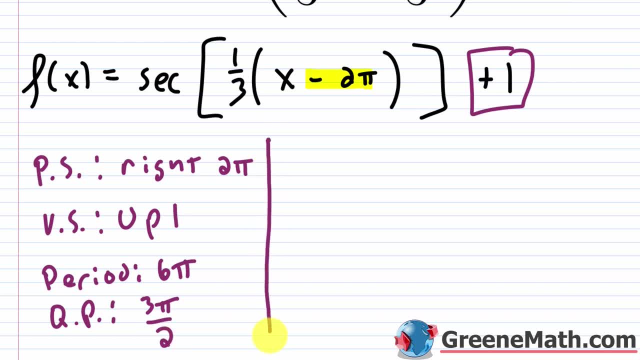 So it's three pi over two. Okay, so if you want to do this using graphing transformations again, typically we always do that for y, But for x it just depends on the student. I'll just give you the information. If you want to do it that way, that's up to you. 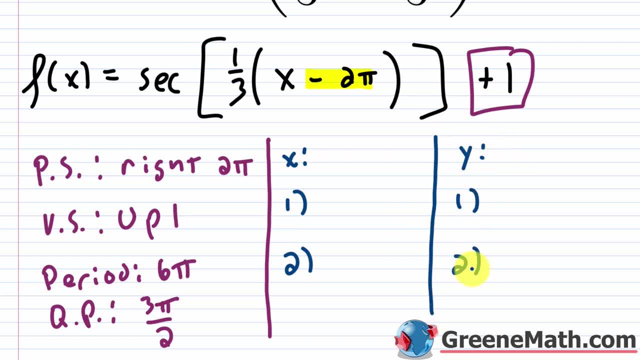 So let me put out x and y here. So for x again, you have to undo what's being done to it, And to do that you go in the reverse order. So, as we talked about in the first problem, this is done. 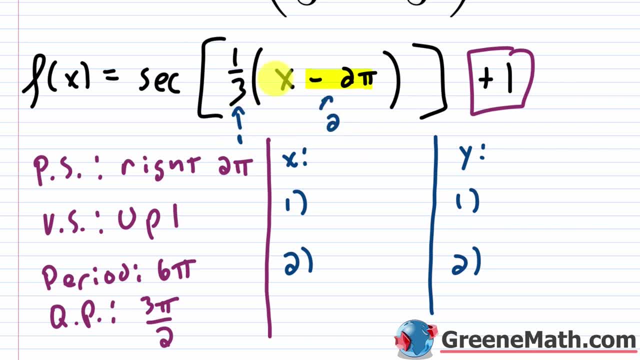 first and this is done second, because you're reversing the order of operations. you go inside the parentheses first, So now this would be second, and you multiply second, So now this would be first, And you have to undo what's being done, So multiplying by a. 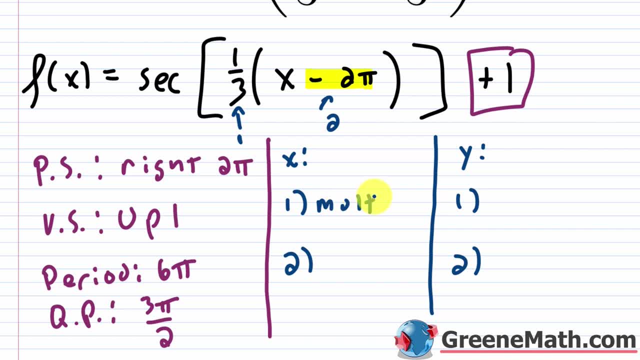 third, To undo that, you need to multiply by three, So multiply by three. And then to undo this subtraction of two pi, you need to add two pi, So add two pi. And so what's happening is this: multiplying by three, that's giving you a horizontal stretch by a factor of three. And 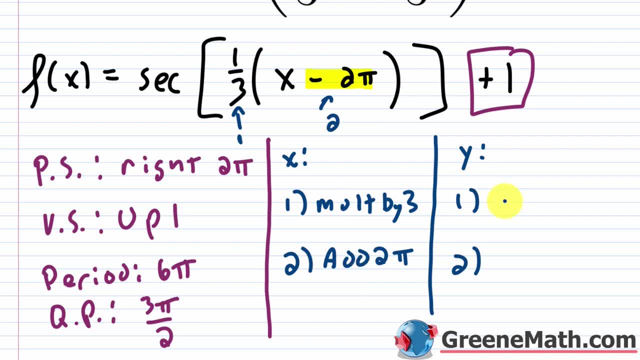 then adding two pi. that's going to shift me to the right by two pi. Then for y again. that's very straightforward. You don't have anything outside here, you can just put a one and a half. So that's going to shift me to the right by two pi. And then for y again. 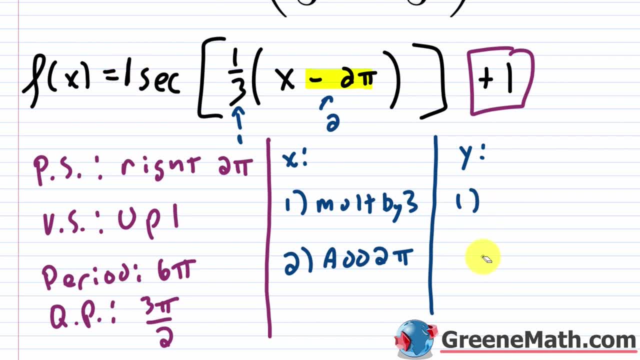 if you want. so really I put one and two, but you just need one thing here, So you wouldn't even consider that, because multiplying by one is not going to change anything. So really all you have to do here is just add one, And so that just shifts me up by one unit. So again, if you want. 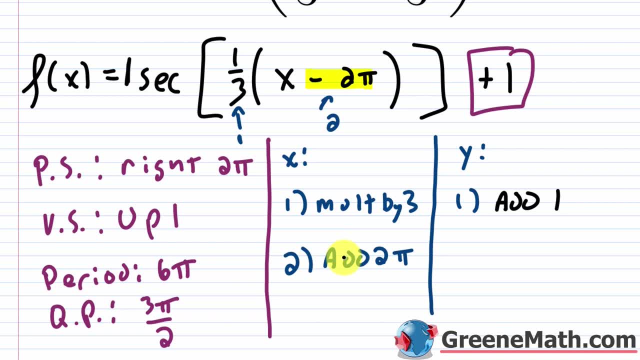 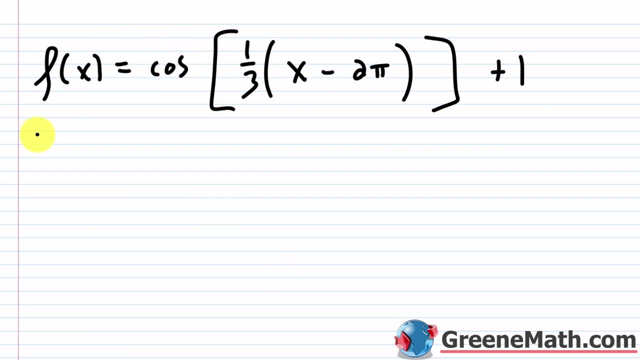 to do it this way. it's up to you. I'm going to use the quarter period method because most students find that easier. So let me go ahead and grab this real quick And I'm just going to erase this and just write in a cosine: Okay, so, going back to the basic points we had, so we're going to say: 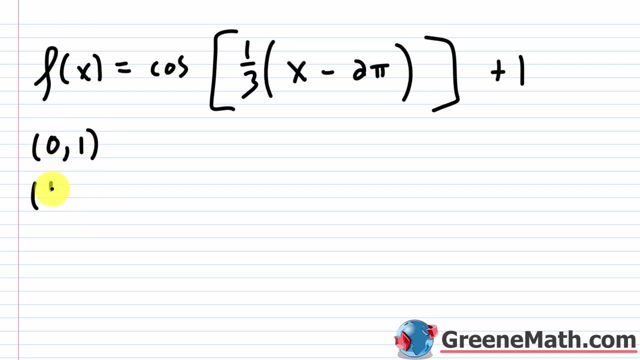 that we have zero comma one, again, starting at the maximum. then you have pi over two comma zero. that's your x intercept. then you have pi comma negative one, so down to the minimum. then you have three pi over two comma zero. so that's your x intercept: you slide. 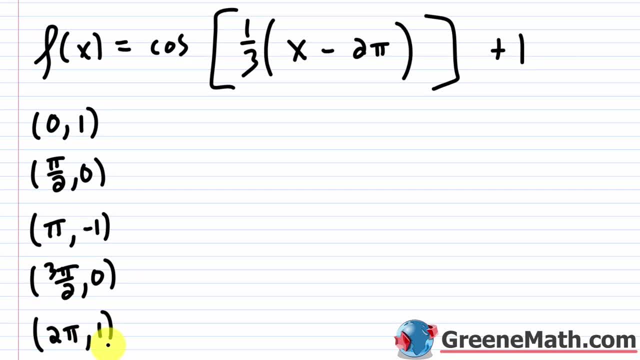 down a little bit and then you'd have two pi comma one, so you're at the maximum for the end of the cycle. So we're going to again. you can use the quarter period method or you can use the graphing transformations that we wrote on the other page. we're going to find the x coordinates. 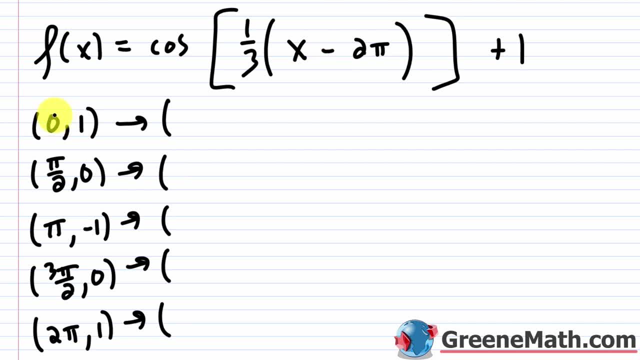 first. So again you would start with a shift, because this guy right here is zero, So you're just going to add two pi, because we're shifting two pi to the right, So this guy is going to occur at two pi now, And then, from that point on, you're just going to add quarter periods, So the period 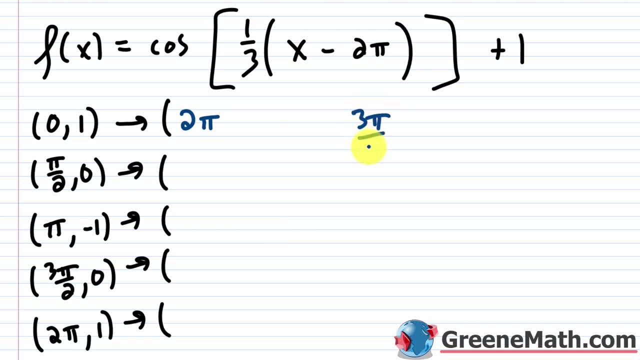 was six pi and the quarter period was three pi over two. So if I add that to two pi, what that's going to give me. let me multiply this by two over two So you could say this is four pi over two. So this would give me seven pi over two. So this is seven pi over two, And then 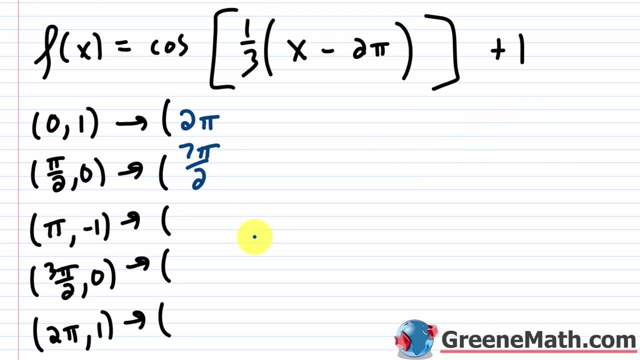 from this point on, you're just going to keep adding three pi over two, So seven pi over two plus three pi over two, that's 10 pi over two. Again, you can simplify that, but we'll do it in a moment. 10 pi over two plus three pi over two, that's 13 pi over two, And then 13 pi over. 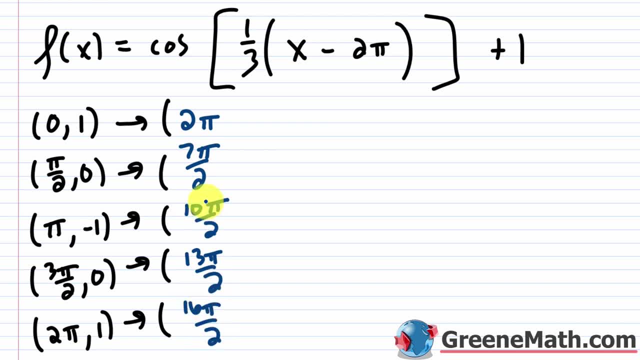 two plus three pi over two, that's 16 pi over two. So this right here would be five pi if you simplified. And then this right here would be eight pi if you simplified. Okay, so now that we have the x coordinates, again for the y coordinate you can just use graphing transformations. 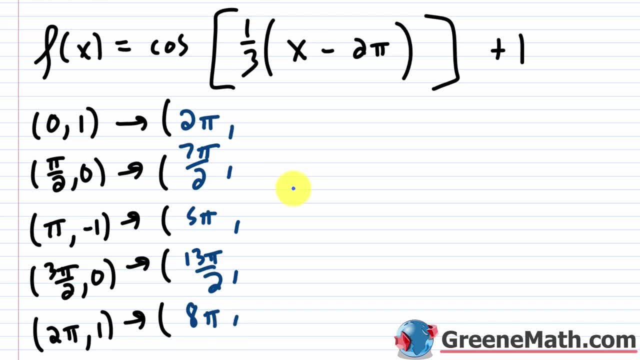 you could plug in if you want, but again, it's the same thing. So what I would do is I would just y coordinate is here. I'm just going to add one because we're shifting up by one unit. So one plus. 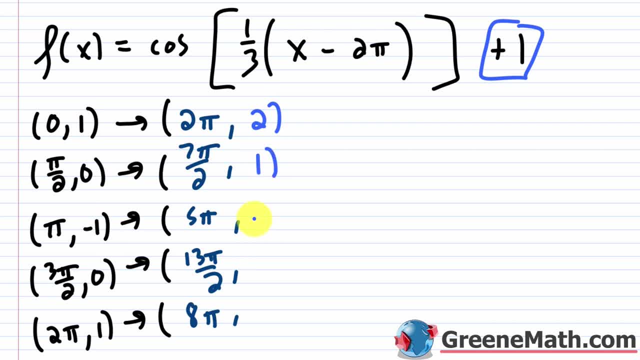 one is two. zero plus one is one negative. one plus one is zero. And again for this one and this one you can just copy. So for zero it goes to one, and then for one it goes to two. And let me paste. 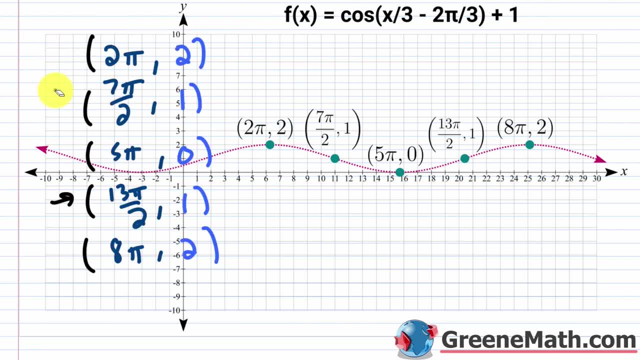 this in Once again. I'll just mention this. I have a link for you on Desmos if you want to follow along more closely. maybe you're having trouble because of the scale of the graph or you're using a smaller device or something like that. But you see, the beginning of the cycle. we have this two. 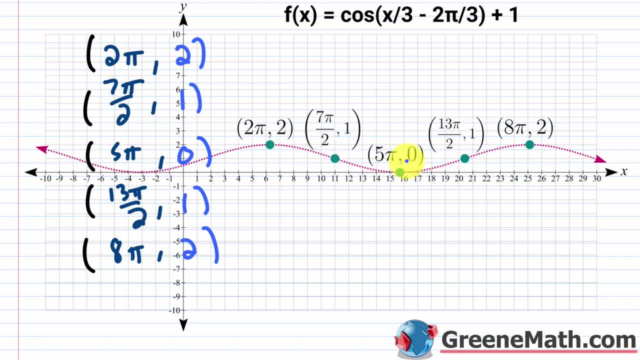 pi comma two, then we have seven pi over two comma two, and then we have seven pi over two comma two, Then we have five pi comma zero, you have 13 pi over two comma one and then eight pi comma two. The common mistake that students make is they're not paying attention And they say: okay, I have. 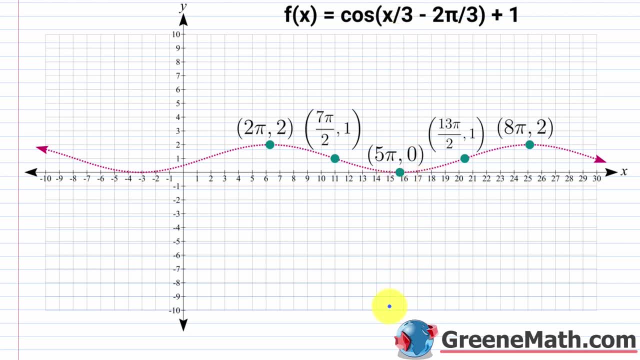 an x intercept here, So they draw a vertical asymptote. That's wrong. You want to look at what happens at the quarter? So at the quarter and three quarters. okay, because this guy has been shifted up by one unit. Again, a lot of teachers will take and draw that new midline. 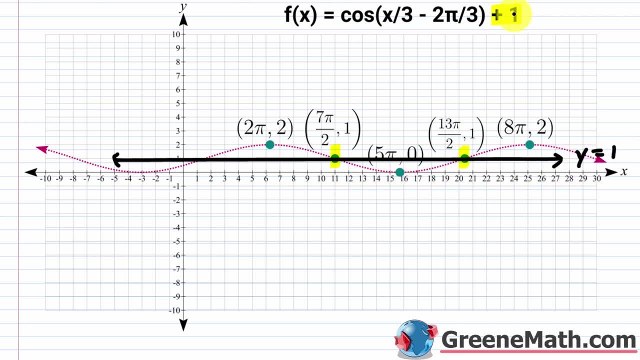 So this is y equals one. normally it's y equals zero or the x axis, But because of the plus one it shifted up by one unit. So this is y equals one. normally it's y equals zero or the x axis. 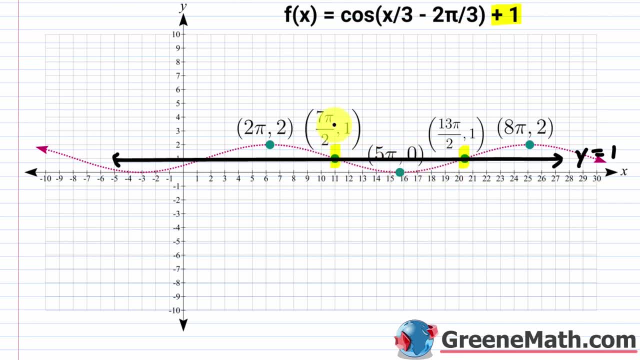 It shifted up by one unit. So whenever you have a point that's on that line, you're going to take the x value there And you're going to say: that's where my vertical asymptote is going to be for the secant function. So x equals seven. pi over two would be a vertical asymptote. x equals 13 pi. 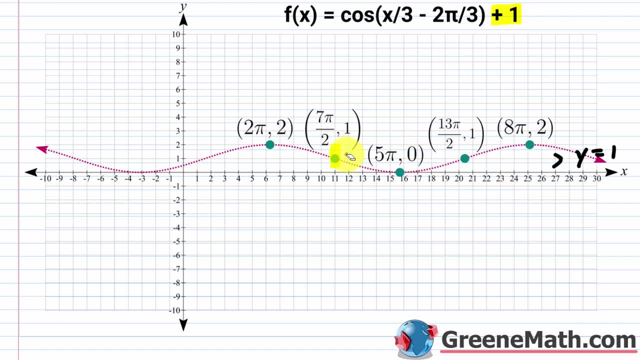 over two would be a vertical asymptote, so on and so forth. Again, if you want to continue this to the left or the right, that's gonna be up to you. Again, you can keep adding quarter periods to your x values to keep going to the right. Remember, the y values are going to cycle. So for the 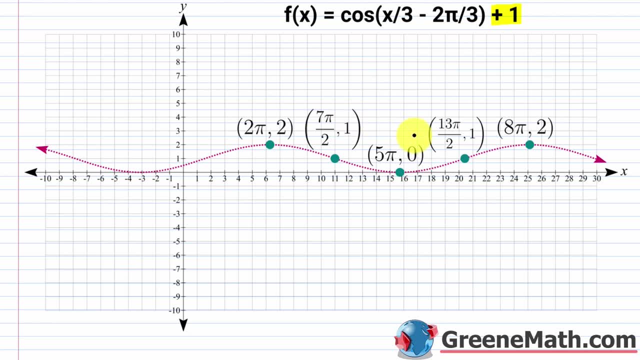 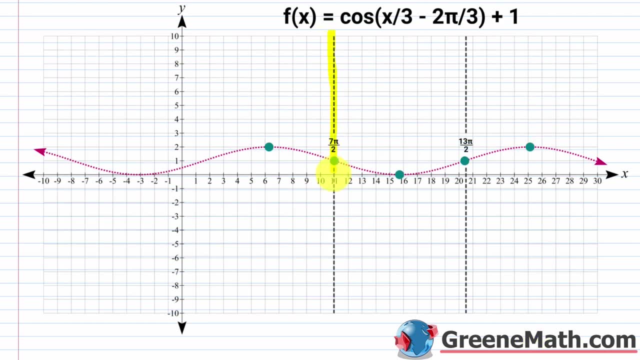 beginning it's two, then for the quarter it's one, halfway it's zero, then for the three quarters it's going to be one, and then finish up at two. Alright, so continuing again. at x equals seven pi over two, you can have a vertical asymptote, And then x equals 13 pi over. 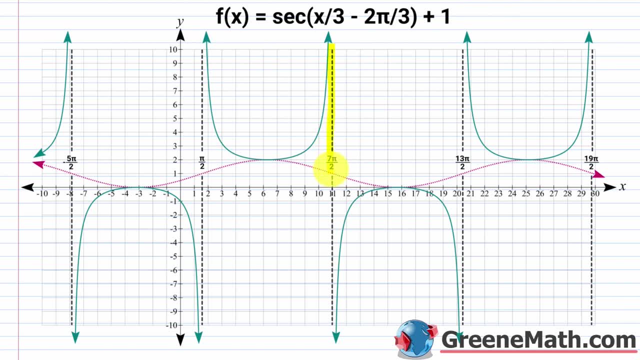 two. you can have a vertical asymptote. Okay. so, coming to the graph, let me just highlight what we just did. So this is your x equals seven pi over two. this is your x equals 13 pi over two. So those are the two vertical asymptotes we found for the secant function And again, all you want. 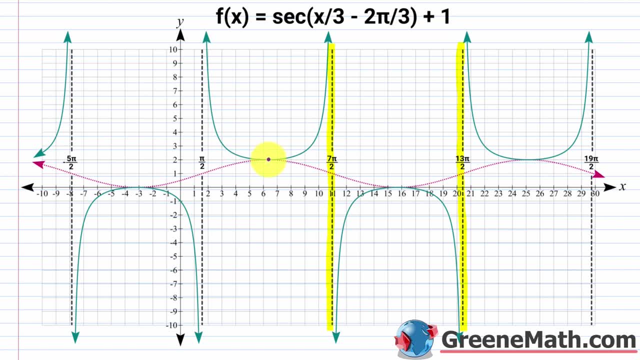 to do is you want to take that point and let's just say it's about right there, And you're going to sketch this to where it approaches the vertical asymptote. When you look at this right here, for the cosine this is a hill, So here it's going to be a valley, So this maximum becomes a local minimum. 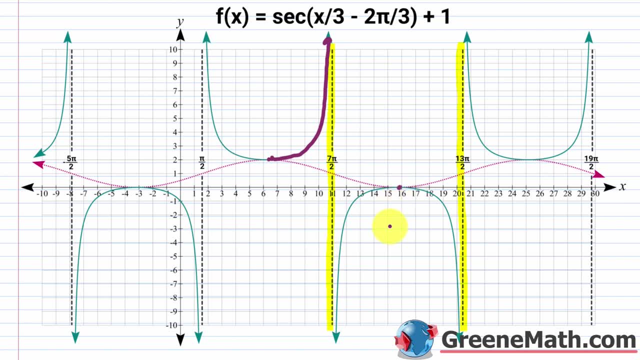 here And then again, similarly, let's say, we make a point about right there And we would say that you could go this guy approaching the vertical asymptote And then this way you would approach the vertical asymptote. So just like that. Again, it does not have to be perfect. 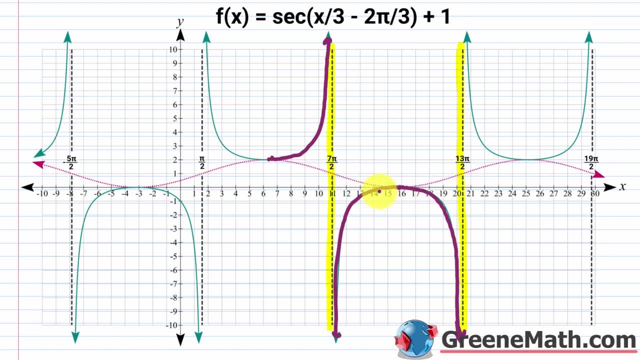 just get it as good as you can. Again. this valley right here on the cosine graph becomes a local maximum on the secant graph. Let's say you have this point about right there that you found. So this guy right here would be drawn to approach the vertical asymptote. 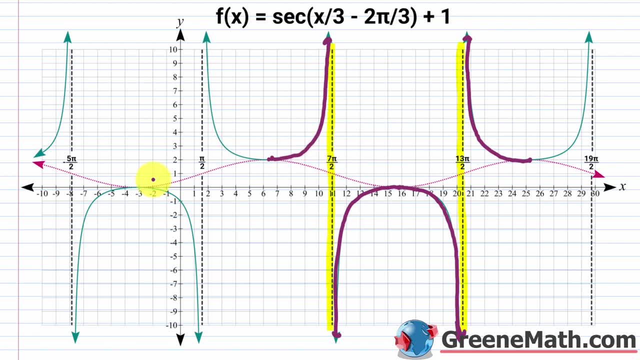 but not touch it Again. if you want to extend this to the right or to the left, you can click the link on Desmos and just practice that way. But generally just drawing one cycle of this guy, particularly if you're self studying- that's good enough. All right, now let's change. 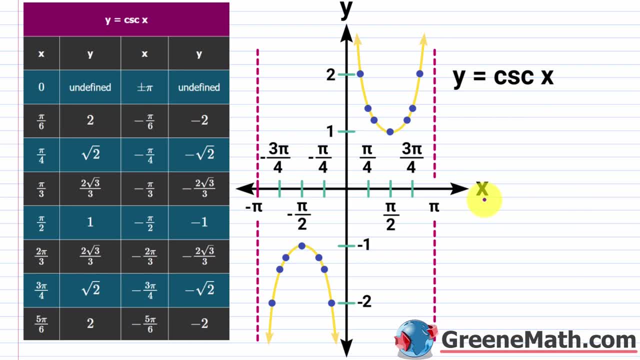 things up and look at the cosecant function. So with this one you're going to see that a lot of things we learned with the secant function is just going to carry over. So let's do: y equals the cosecant of x. And again, I'm going to do this over one period. Now, negative pi and pi will not. 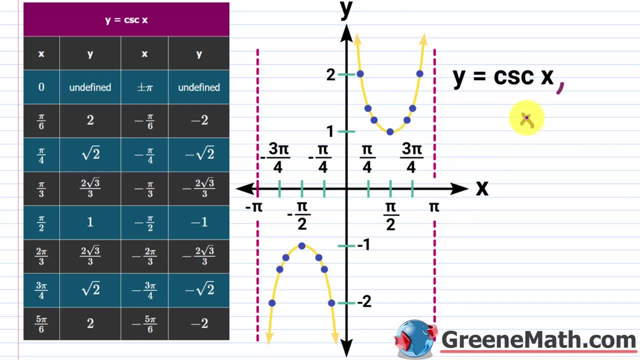 be included here because that's going to give you undefined. So let's say that x is strictly greater than negative pi and strictly less than pi. So let's think about this using the unit circle and come back up here for a moment. So remember that the cosecant of x, by definition, is one over. 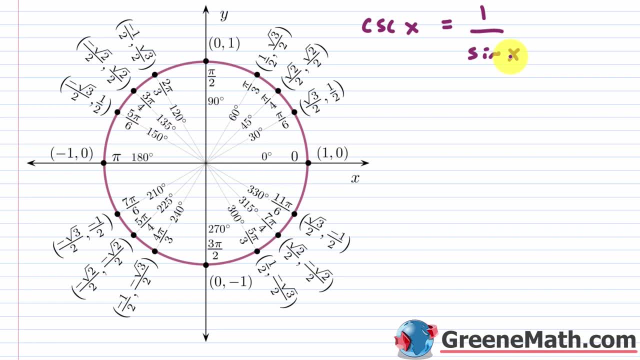 the sine of x. So a moment ago I said that it would be undefined at negative pi and pi, But just thinking about where the sine value is zero. so that's right here at zero, right here at pi, So just using the standard unit circle. But again, 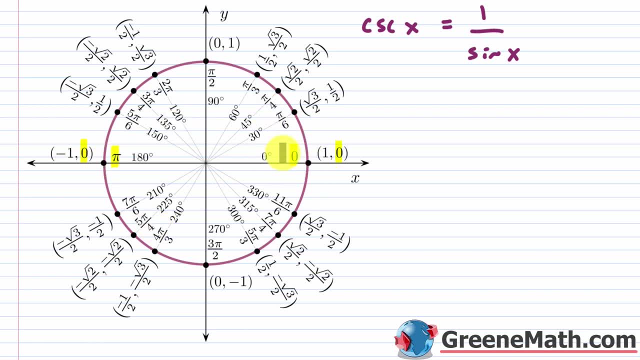 this is going to repeat every pi, So you have zero pi, two pi, three pi, four pi, five pi, so on and so forth. Or if you wanted to rotate clockwise, you could say: let me just show you this real quick: If you rotated like this, this would be negative pi, So that is negative pi. 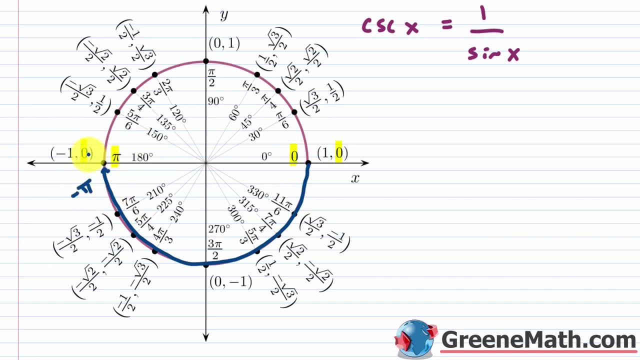 that is coterminal with pi, So it's the same sine value. So you could do negative pi, negative two pi, negative three pi, negative four pi stuff like that. you're still going to get undefined value for cosecant because the sine value is zero. So going back you will see that. 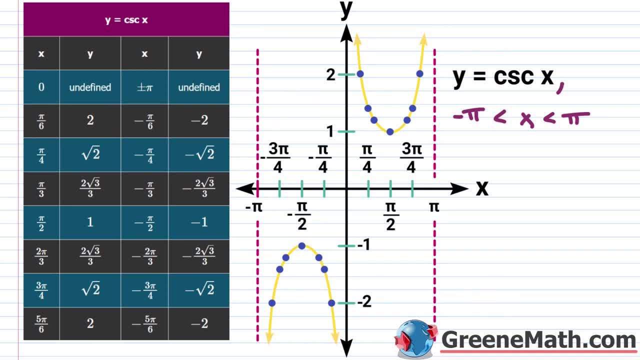 anywhere where the sine value is zero, you're going to get these vertical asymptotes. So again, at negative pi you're going to get one. you get one at zero. but you typically do not put a dash line right there because this is the y axis, So you can put one in if you want. just know that. 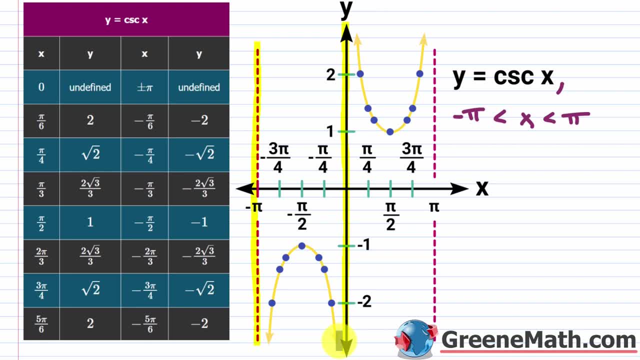 that is a vertical asymptote. So it would be x equals zero, or again the y axis, and then here you have pi. But if you keep going you'd have two pi, three pi, four pi, five pi, six pi, six pi. 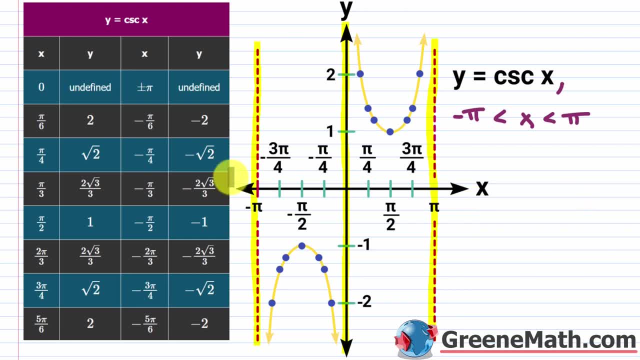 four pi. if you kept going this way, you'd have negative two pi, negative three pi, negative four pi, so on and so forth. So you can basically say this is going to happen at pi n where n is an integer When you look at this point right here, so this point right here, you have a y value of 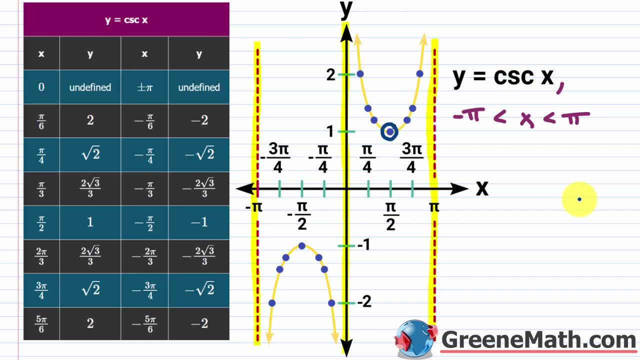 one. So this will be a shared point for cosecant and also for sine. And then here you have a y value of negative one. that'll be a shared point for cosecant and for sine. I'll show you that when we get to the combined graph. So just remember this point right here. this is going to be pi over. 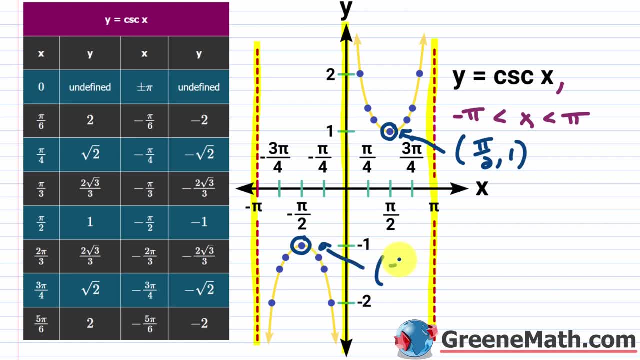 one. and then this point right here, this is going to be negative pi over two. Remember that's coterminal with three pi over two and then comma negative one. So again, just thinking about the behavior of this guy as you go from pi over two for that x value where the sine value is one, 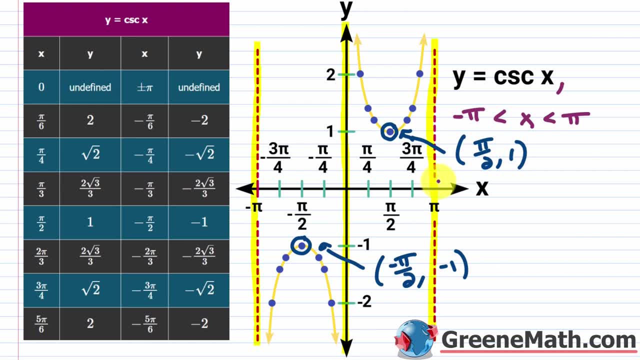 to an x value of pi where the sine value is zero. well, again, because the cosecant of x. let me write this out: because the cosecant of x is equal to one over the sine of x. well, the value here. as you go this way and you get closer to an x value of pi, it's getting 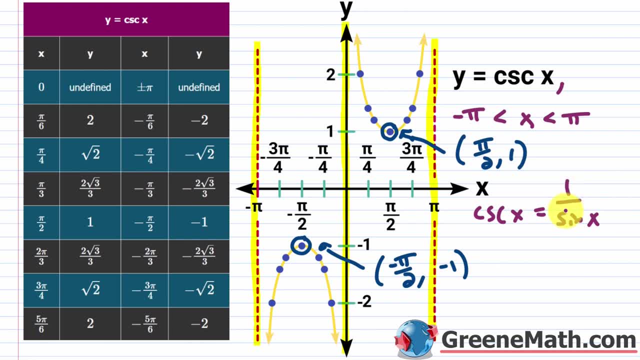 closer and closer to zero, but it's never going to touch it. So one over something that's really really close to zero again, this is going to blow up and we say: this increases without bound, or it's approaching positive infinity. Then, similarly over here, if you. 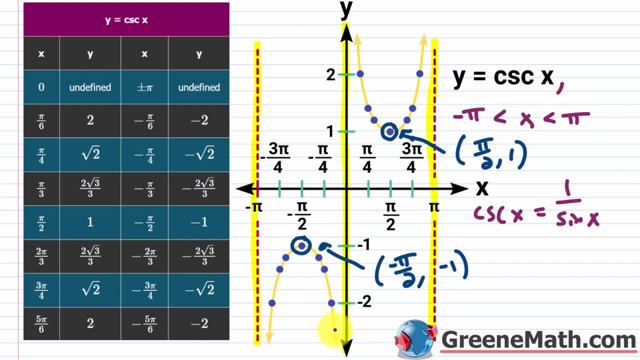 follow this part right here you're going to decrease without bound or approach negative infinity. So, just like we saw with the secant function, same process is happening. it's just happening at different places on the graph. Now we can go through a few basic. 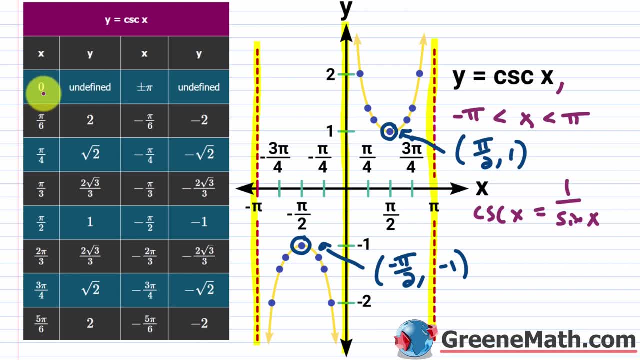 points. this is just something you can read through for reference. So if the x value is zero, again y is undefined. this is also going to happen at plus or minus pi. you would get undefined Again. this is pi n, where n is an integer, because you have a sine value. 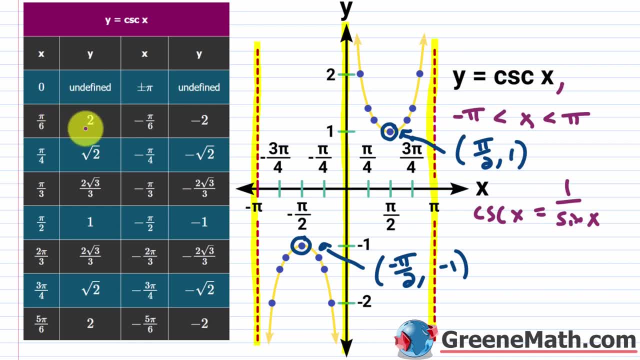 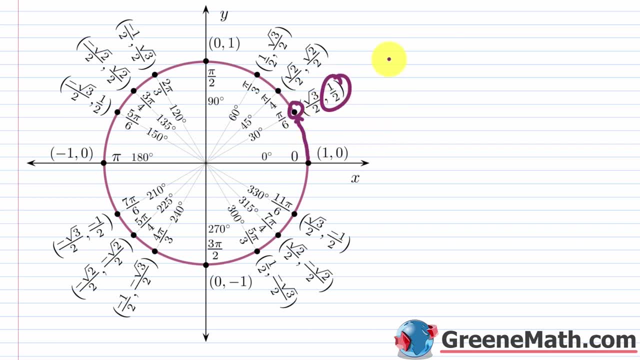 of zero. Then when you think about something like pi over six, you get two Again. just to show you that one, just so this is crystal clear. if you look at this right here, this is pi over six. well, the sine value is a half, So the cosecant of pi over six is one. 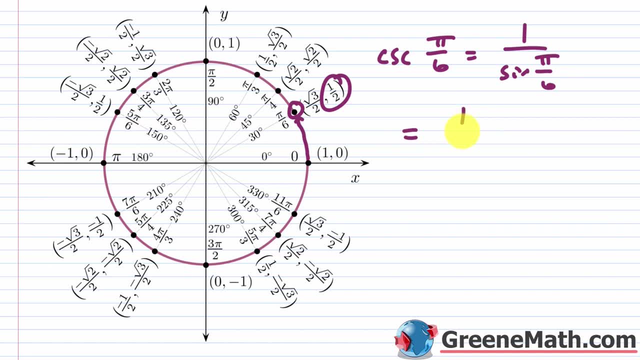 over the sine of pi over six, which equals one over one half, which again is two If negative pi over six. I'm rotating clockwise, So we saw that earlier And so this is coterminal with 11 pi over six. But the thing is cosecant and sine they are negative in quadrant four. 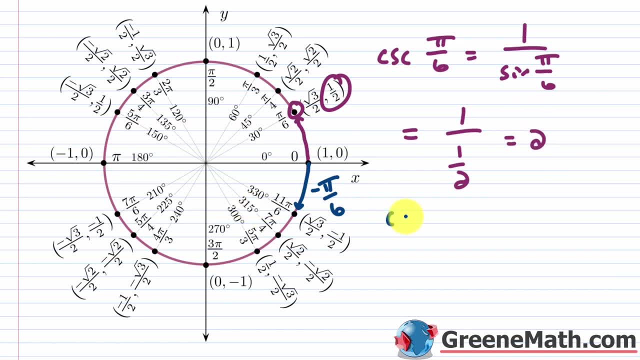 So that means I'm going to get the opposite of this. So I would want negative two. So the cosecant of negative pi over six is equal to one over the sine of negative pi over six, which is equal to one over negative one half. Again, you can take that y coordinate right. 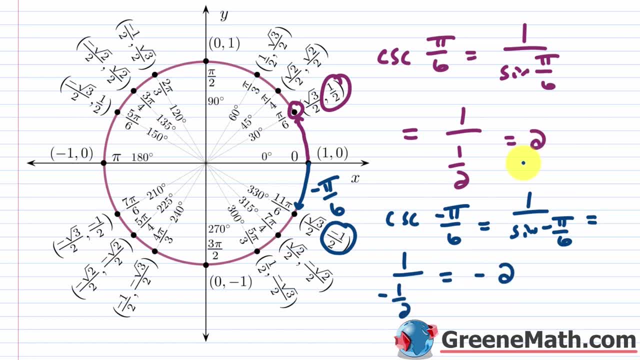 there, And so this is equal to negative pi over six. I get minus 16 over twice. pi over three over three. I would just take the two on the real on that here. So the cosine of negativeimyof one half y parallel here. 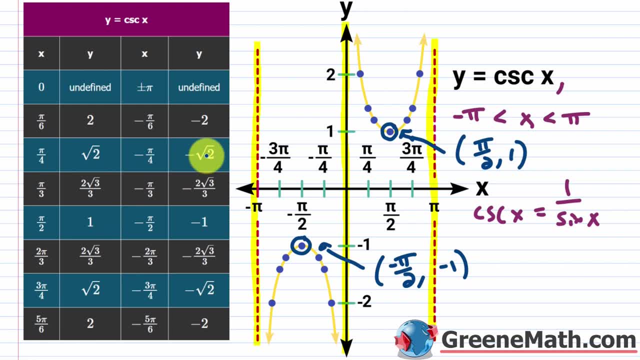 So here we come. Ukraine, That sections. Then if you're putting three squares in the square, that's with negative pi minus 19. Then you can give minus 19 times the square over two. What's calling the��maker Three plus five times three over three. This is: 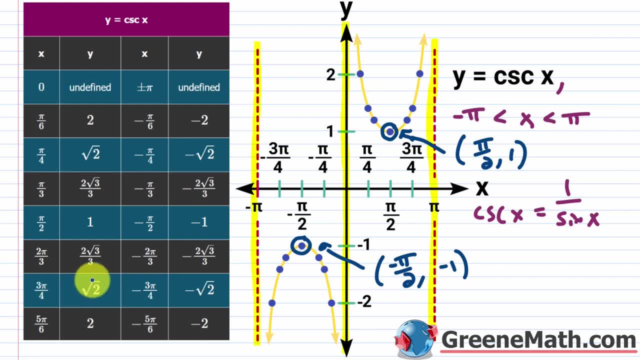 the cosine of three two times square through. So to think about a video over pixels per square over six is a miscelline. So we can just do the detection case to express that we're going to get two square over two- 5 or 6, you get 2.. And negative 5, 5 or 6, you get negative 2.. So just like we saw with secant. 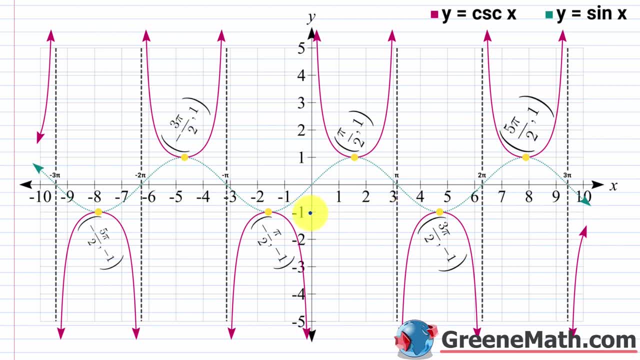 and cosine. we're going to use the sine function as a guide when we graph cosecant. Again, where there's a y value of 1, you're going to have a shared point. Where there's a y value of negative 1, you're going to have a shared point. So you're going to use those shared points Again when you 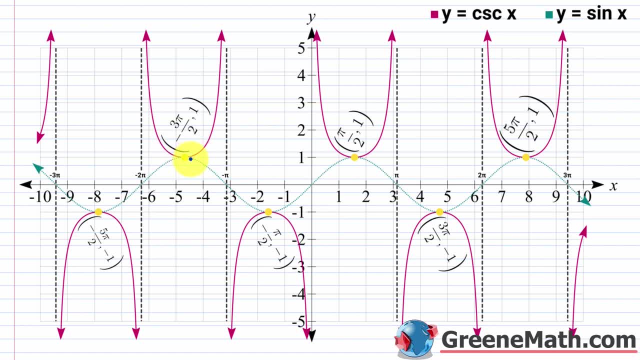 have a hill here, you're getting a valley here. So this maximum. here again, the range for sine is the same as the range for cosine. It's from negative 1 to positive 1, with both being included. So whenever you have a y value of 1, you're at a maximum on your sine graph. So a maximum here. 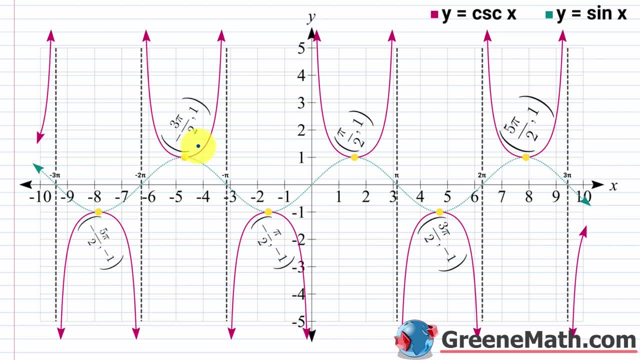 gives me a local minimum. here Again, there is no minimum or maximum for the cosecant function or the secant function, but you do have those local minimums and local maximums. Some books call that the relative minimum and the relative maximum, if you're used to that terminology. 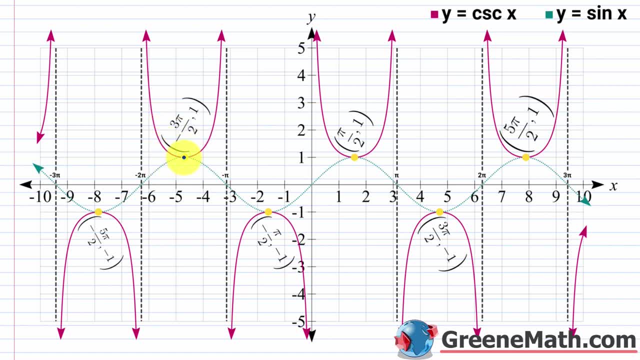 But this hill right here becomes a valley here, where you could say: this maximum here becomes a local minimum here, Then this valley right here becomes a hill here. So in other words, this minimum here becomes a local maximum here, and so on and so forth. Then again the other thing: I 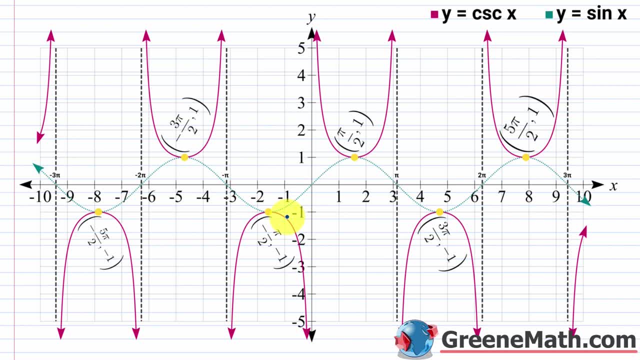 would call your attention to is that in this form, because there's no vertical shift. when you look at where you have the x-intercepts on your sine graph, that's where you're going to have your vertical asymptotes for the cosecant graph. So something like pi, you would also have 0.. Again. 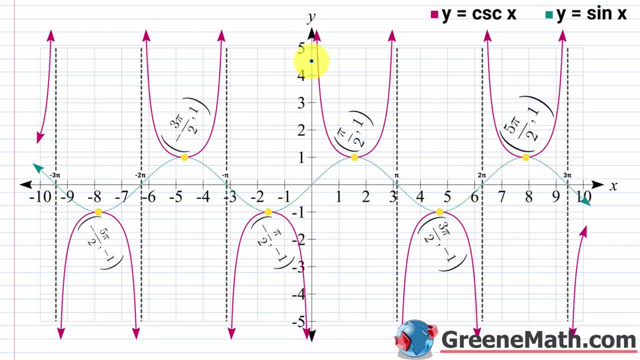 we typically do not draw that in for the y-axis. If you want to, it's not wrong, But you would have 0, pi, 2pi, 3pi again going over here, negative pi, negative 2pi, negative 3pi, so on and so forth. 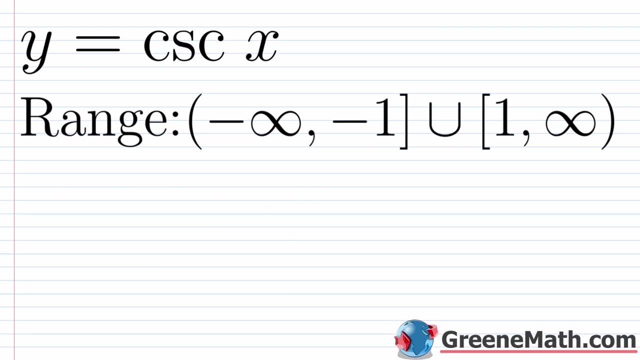 So, just like we saw with the secant function here is going to be from negative infinity to negative 1, where that's included, and the union with 1 going out to positive infinity. So you don't have any y values between negative 1 and. 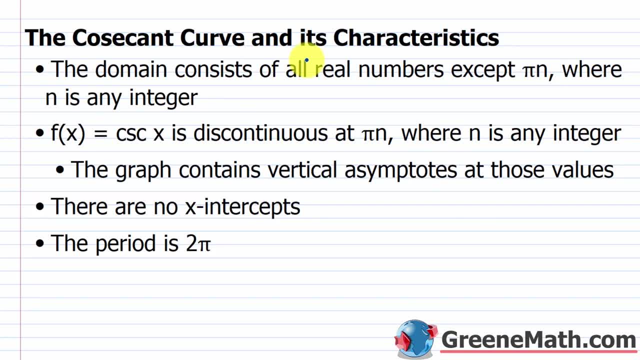 positive 1.. All right, let's spend a little bit of time looking at the characteristics of the cosecant curve. So we have here that the domain consists of all real numbers except pi, n, where n is any integer. Again, that's because the sine value would be 0 there, and so your cosecant. 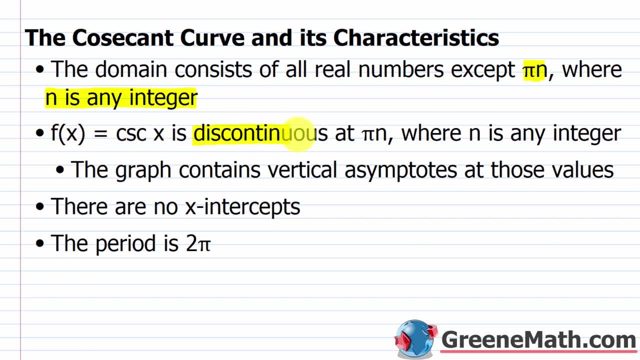 function would be undefined. We have f of x equals cosecant of x is discontinuous. Again this pi? n where n is any integer And the graph contains vertical asymptotes. at those values There are no x-intercepts. You're. 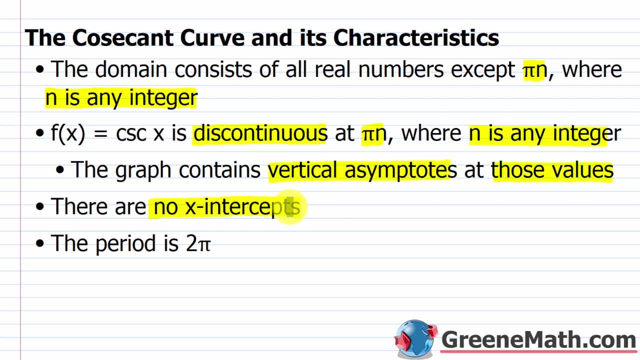 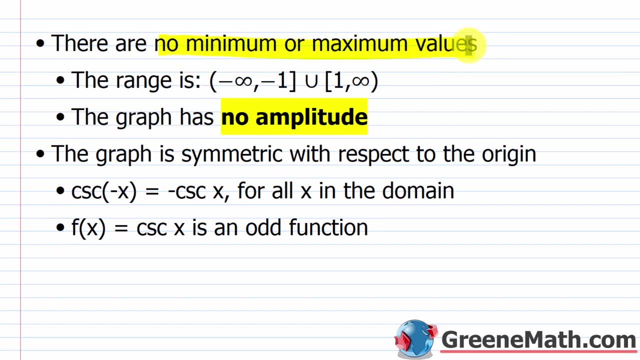 only going to get those when you start shifting the graph up or down. But on the standard y equals cosecant of x. there are no x-intercepts. The period is 2pi. There are no minimum or maximum values. Of course we have those local minimums and local maximums that we use to sketch the 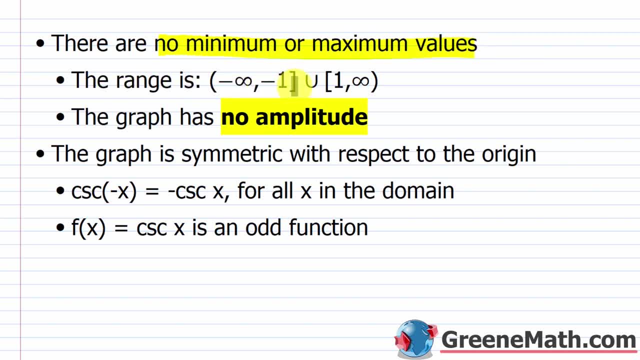 graph. The range is from negative infinity to negative 1, with this guy being included and the union with. you have 1 to positive infinity, again where 1 is included, but you don't have any y values between negative 1 and positive 1.. So keep that in mind. The 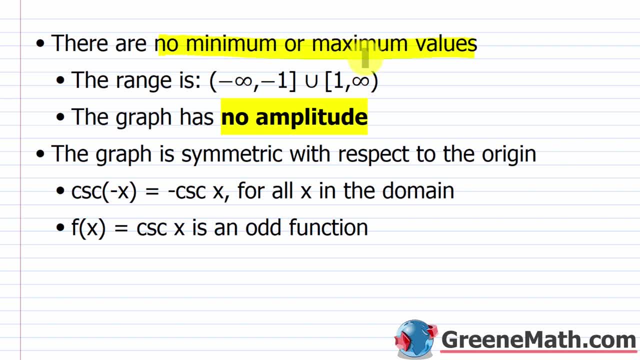 graph has no amplitude because, again, there are no minimum or maximum values. You're just going to see amplitude when you work with cosine and sine. Now the graph is symmetric with respect to the origin, So the cosecant of negative x is equal to the negative of 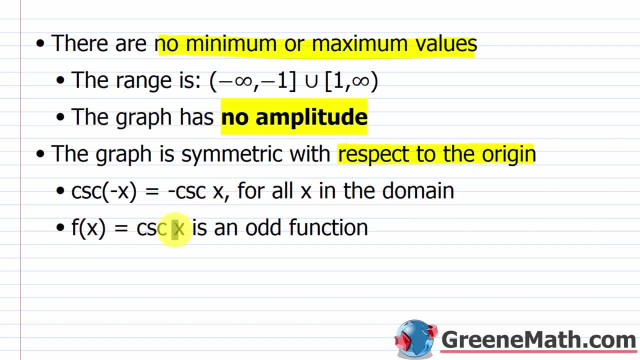 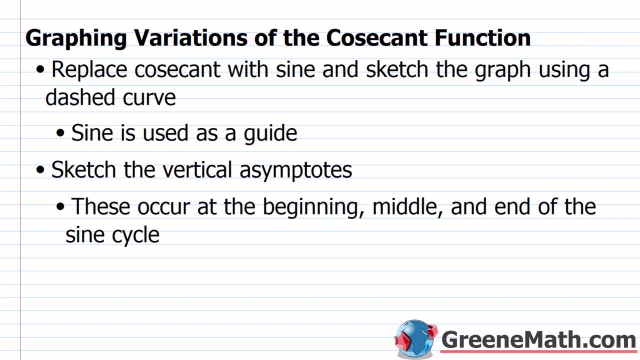 the cosecant of x for all x in the domain. So f of x equals the cosecant of x is an odd function, so just like the sine function. Alright. so now let's talk about graphing variations of the cosecant function. So this is pretty much the same thing as we saw with 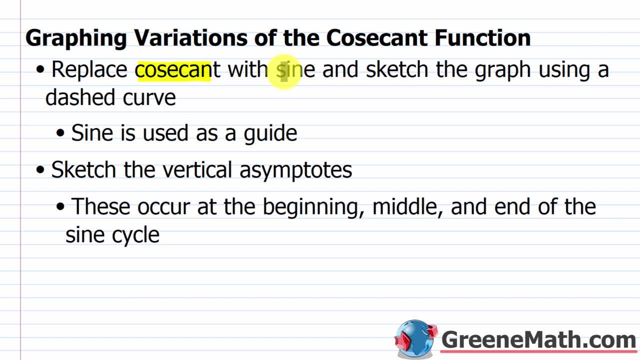 the secant function directions. So we're going to replace cosecant with sine and sketch the graph using a dashed curve. That's your guide function. Sine is used as a guide. Sketch the vertical asymptotes Again when you think about this, because you have vertical shifts. 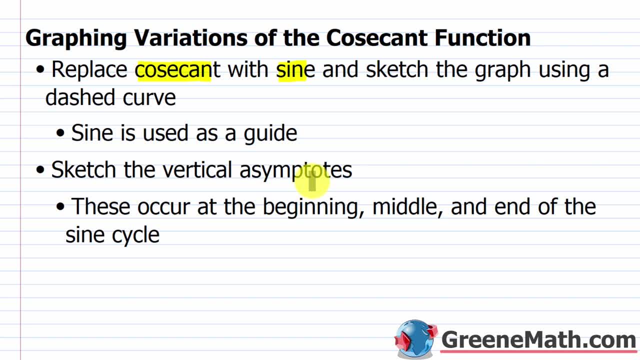 you cannot just say that the vertical asymptotes will occur wherever the x intercepts are on the sine graph that you're using as a guide. That will only work if you don't have any vertical shifts. So what I always teach people is they occur at the beginning, middle and 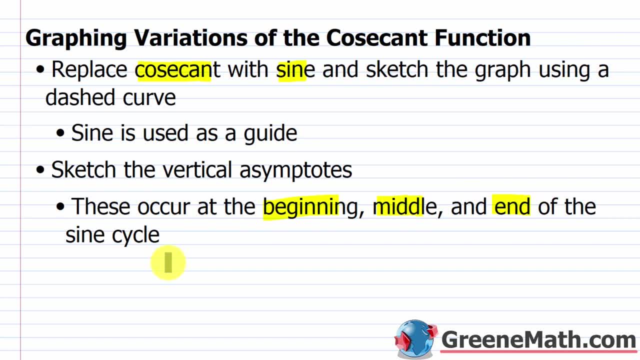 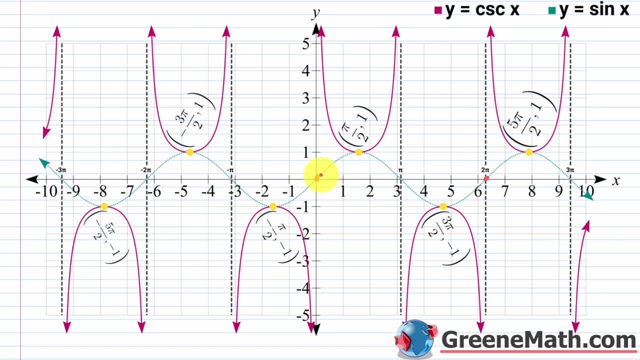 end of the sine cycle Because, remember, on your normal sine graph you have- let me just come back to this for a moment- so your cycle is going to go from right here to right here, so from 0 to 2 pi. 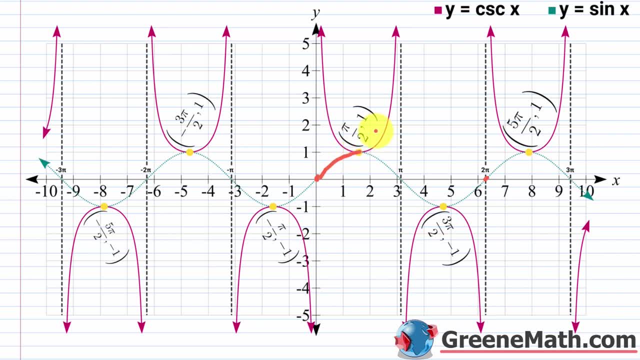 You're going to start out at an x intercept, You're coming up to the maximum and then you're coming back down to an x intercept. so, right there, Let me do that in a different color And actually let me mark this one and this one, and this one in a different color. 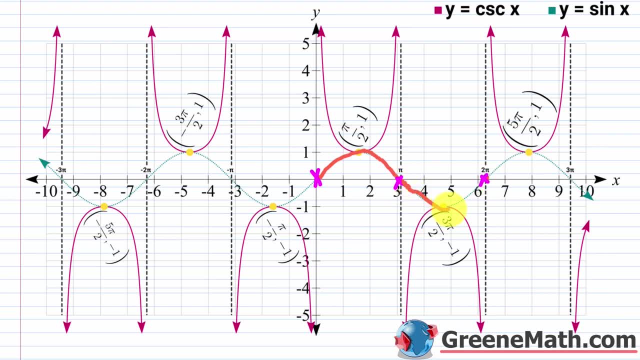 I'm going to go back to this one, So let me come down. so you're going down to the minimum and then you're coming back up to the end of the cycle, which is an x intercept. So the beginning, the middle and the end. 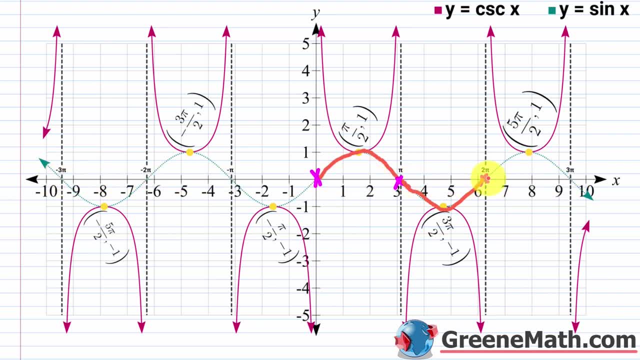 If you remember that this midline is y equals 0, so you're on the x axis. if you had something like a vertical shift up by 1,, well then that midline is going to be y equals 1.. If it was, 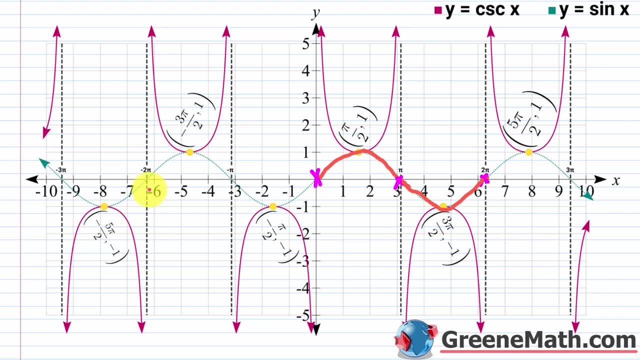 let's say a shift down by 4, well, now it would be: y equals negative 4.. So a lot of people will draw that midline in. You can do that, But what I always do is just say, okay, what point am I going to have? that's first, third and fifth. So at the beginning, 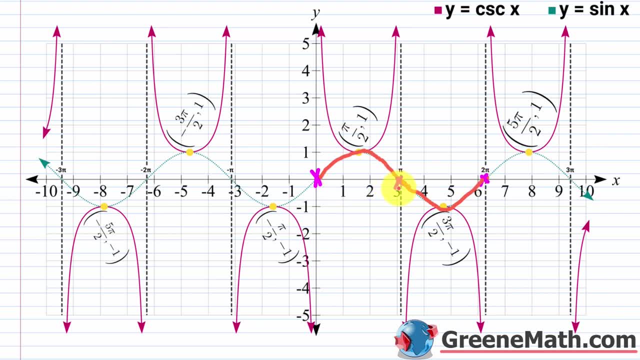 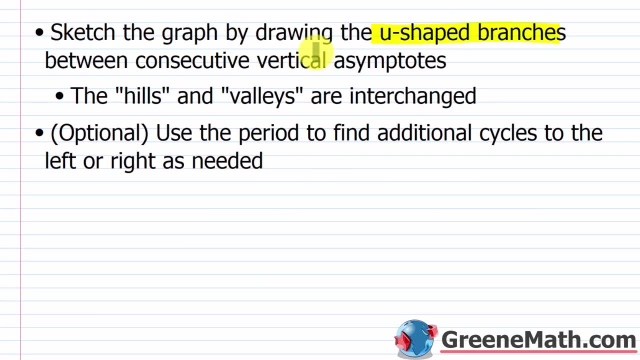 the middle and the end. that's where I'm going to take those x values and draw my vertical asymptotes for the cosecant function I'm working with. All right, then I have sketched the graph by drawing the u-shaped branches between consecutive 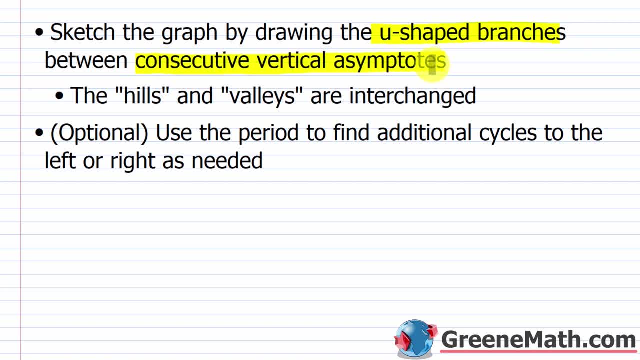 vertical asymptotes. So these guys are going to approach the vertical asymptotes but not touch them. And we have here: the hills and valleys are interchanged And then, optional, I have used the period to find additional cycles to the left or right as needed, If 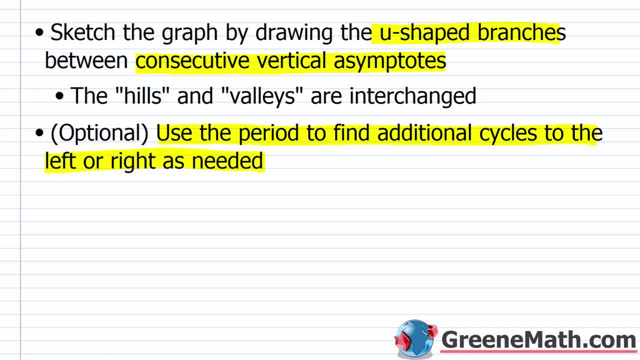 you're self-studying, I recommend just doing one period. You can, of course, just look on Desmos and see it to the left or right as much as you want, But if you're getting this from a teacher as an assignment, they'll generally tell you: well, I want you to sketch. 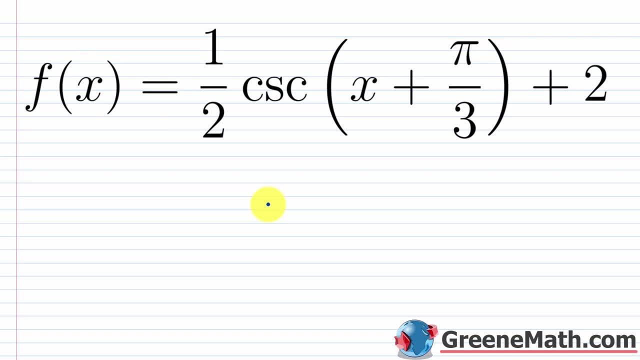 it over this interval. So just follow that. All right, let's take a look at an example. So we have f of x equals 1 half cosecant of x, plus pi over 3 and then plus 2.. So normally I would factor this so I can get the phase. 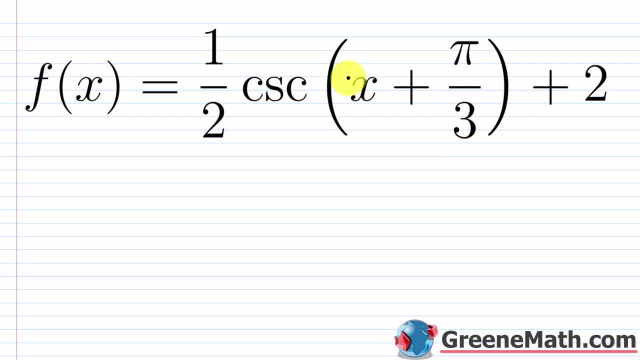 shift. But here the coefficient on x is 1, so you don't really need to factor anything. You can immediately just get the phase shift and say that we're going to go left by pi over 3.. Again you've got to undo what's being done to x. You have plus pi over 3, so that 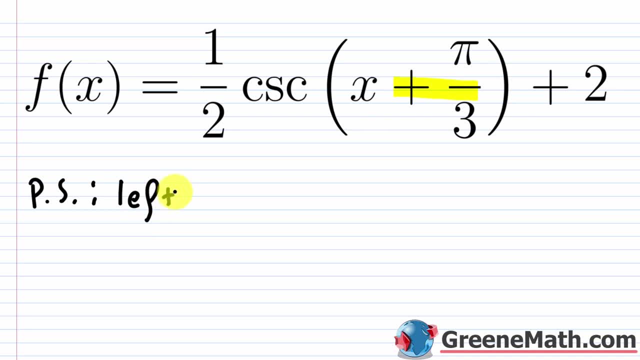 means you need to do minus pi over 3.. So that tells me I'm going left pi over 3.. And then, in terms of your vertical shift, you're going to have plus 2 here. So that means I'm going up 2.. So if you wanted to graph a horizontal line through the middle, 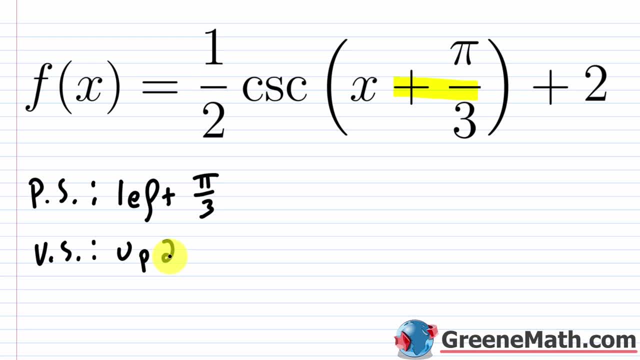 of that guy when you're graphing the sine function as a guide you would sketch y equals 2 for that, Because normally it's y equals 0, and this has shifted me up by 2 units. So for the period it's just the standard 2 pi. So you take 2 pi and you divide by the. 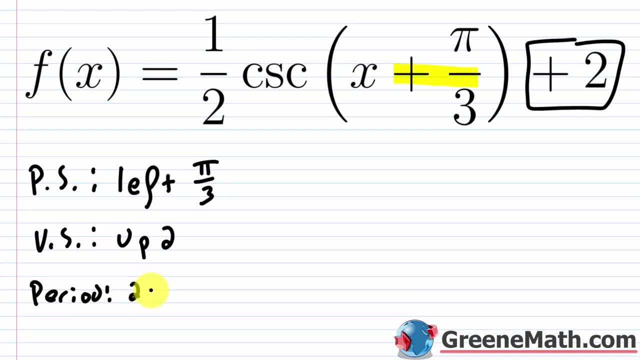 coefficient of x, And so in this case that's 1, so it's just 2 pi, And then the quarter period. if you're using that method, well, it's just going to be 2 pi over 4, which would 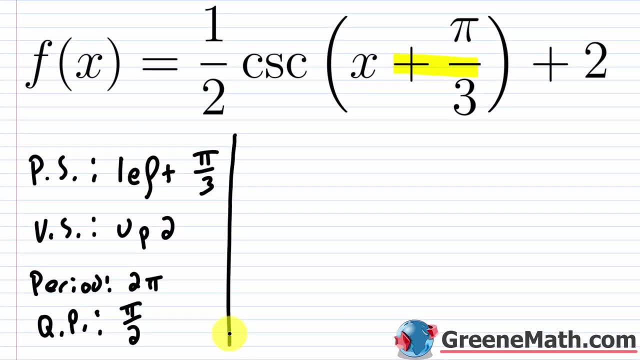 be pi over 2.. So if you want to use graphing transformations, then let's just put down for x. here you only have one thing you'd have to do Again. you're just shifting to the left by pi over 3. So 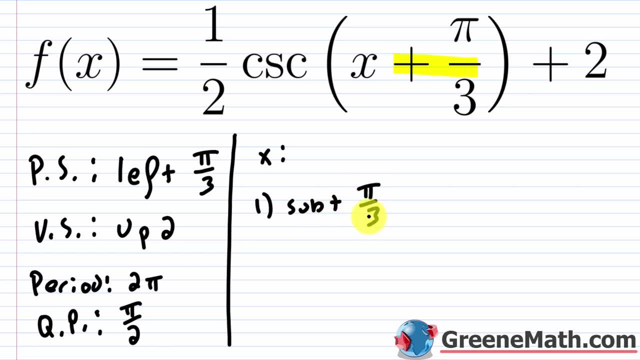 you would just subtract away pi over 3. And that's from each x value, from your standard points for the- and we're going to work with the sine function in a moment when I swap this out. so for the sine function, And then, in terms of the y, you have two things. you 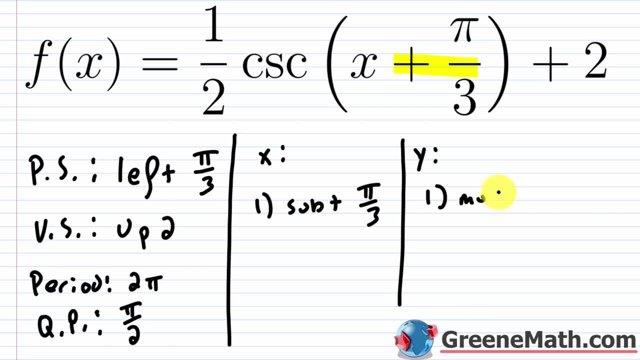 need to do. Let me put a little border here. The first thing is you multiply by half, You multiply by one half, And the second thing is you add 2.. So we're going to use this. If you want to use this, that's up to you. In this case, I think it's probably equal. 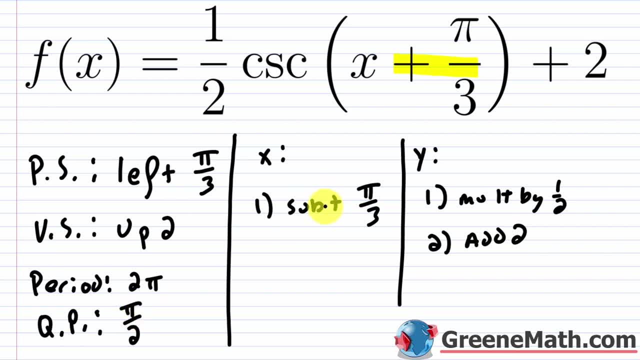 time to using the quarter period method, but a lot of people do not like using graphing transformations for x, for whatever reason. So, thinking about this, this gives me a shift to the left by pi over 3.. This right here gives me a vertical compression by a factor. 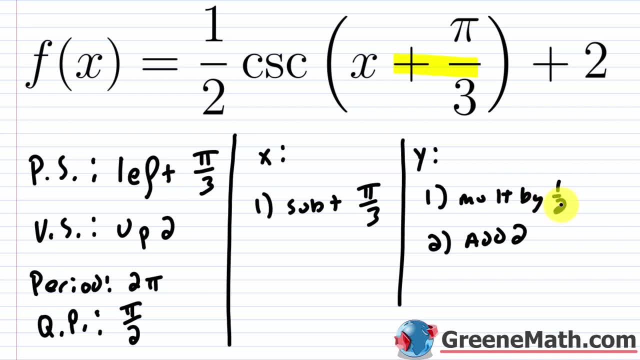 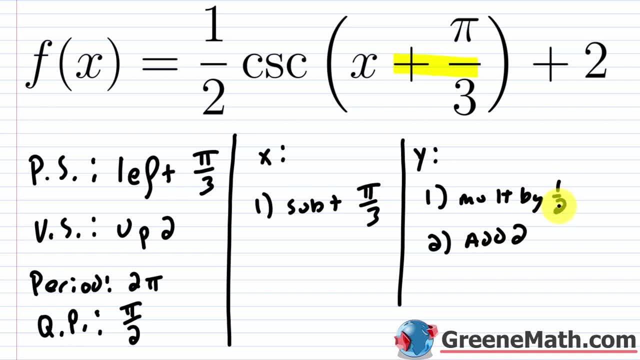 and do that. So I'm going to go ahead and do that. So I'm going to go ahead and do that. Just understand that you're either dividing by 2 or you're multiplying by half for each y-coordinate, Then you're going to add 2.. That's shifting me up by two units And come. 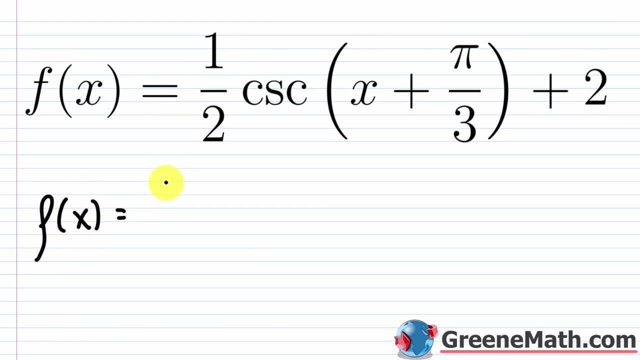 down here and paste this in, so I have some room. So I'm just going to rewrite: f of x equals one half sine of x plus pi over 3, and then plus 2.. Okay, let me get rid of this, Move this up, And we just need to get our points. So just start with your standard points. 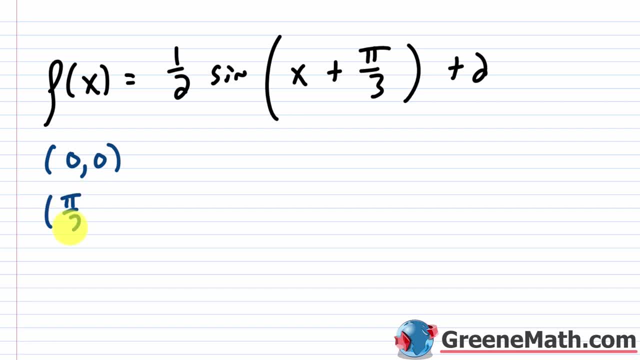 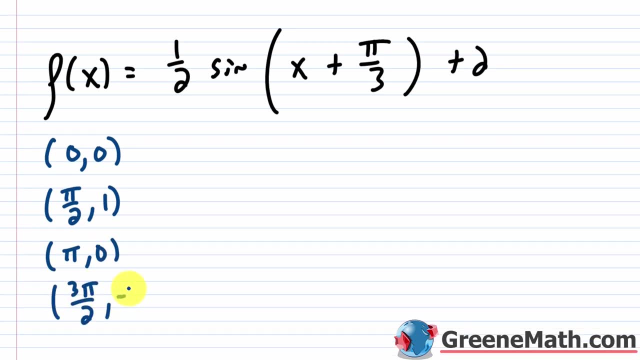 for sine. So you have 0,, 0.. You have pi over 2 comma 1.. Then you have 2,, 2,, 2.. And then pi comma zero. you have three pi over two comma negative one, and then you're going to finish up. 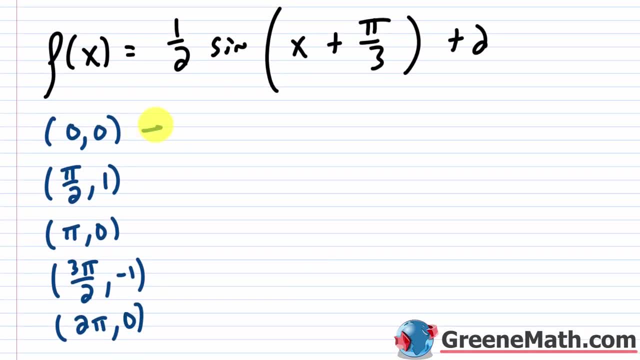 at two pi comma zero. So all you have to do is start things off with your phase shift. So that is going to be minus pi over three. So you take zero subtract away pi over three, So that gives me negative pi over three. Once I've done that, I'm just going to add quarter periods, That's all. 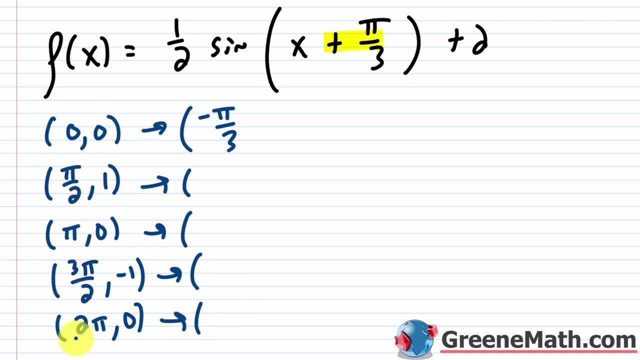 I need to do So again. if you're using this method, you're not going to touch any of these x values. You're only going to do that if you're using the graphing transformations method, And I know that gets confusing. but essentially you're just saying: okay, well, the quarter period here. 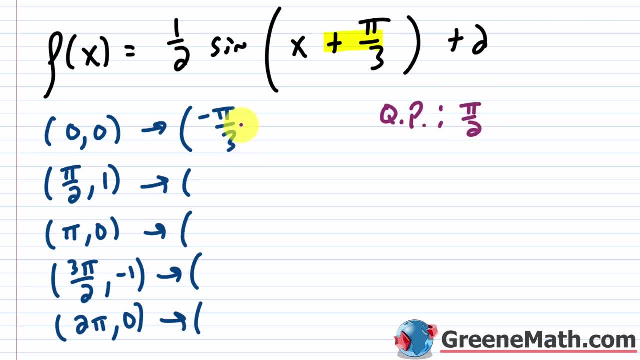 is going to be pi over two. I need a common denominator. Let me multiply this by two over two. Let me multiply this by three over three, So that would give me three pi over six. So three pi over six, and this would be negative two pi, So negative: two pi over six. You can erase this. 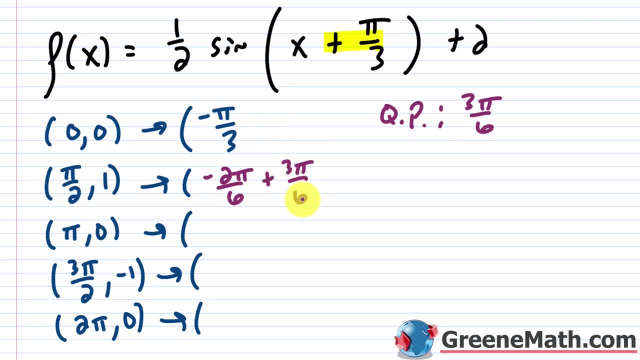 now. So I'm going to add three pi over six, So that gives me pi over six. So this is pi over six. And again, you're just going to keep doing this. So you're just going to keep adding three pi over six, So that gives me pi over six. So again, you're just going to keep doing this. 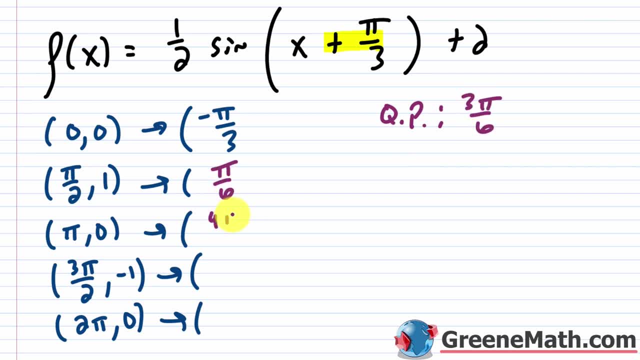 Pi over six plus three pi over six, That is four pi over six. Don't simplify yet. Four pi over six plus three pi over six, seven pi over six, seven pi over six plus three pi over six, 10 pi over six. 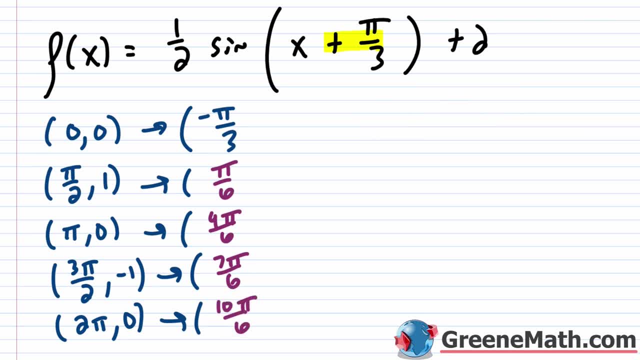 Okay, So now you can simplify. You just want to make sure you're not simplifying. Then you got to get a common denominator again. So four pi over six. four divided by two is two, and six divided by two is three. So it's two pi over three. And then 10 pi over six. 10 divided by two is five. 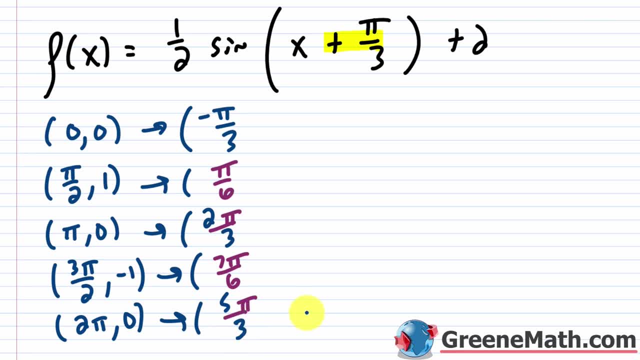 and six divided by two is three, So that's five pi over three. The other way you could have done this. we only have one thing we're doing to x: We need to subtract away pi over three. So if you're using that method, you're working off of these values only. So zero minus pi over three, negative. 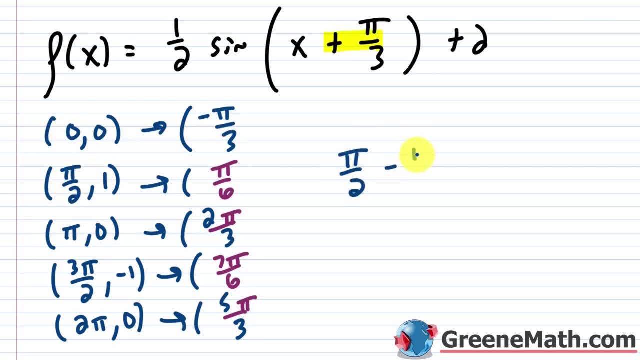 pi over three, Pi over two. let me show you this real quick. So pi over two minus pi over three. Let me make that better here. That's going to give you pi over six. So if I multiply this by three over three, multiply this by two over two, I would have three pi minus two pi, And this is over six. 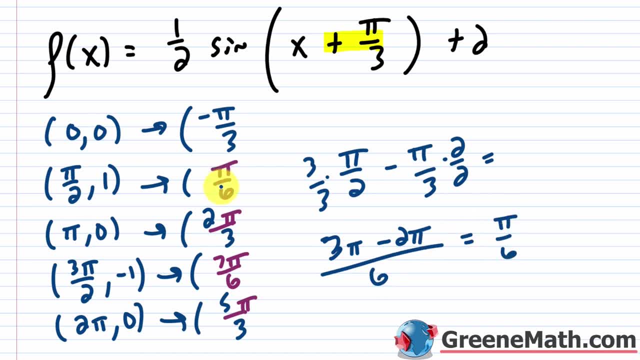 And of course that is pi over six, Same thing as I got right there, And you can keep doing this. if you want, You could do pi minus pi over three. Let me just do one more of them, Just so this is crystal clear how you can use the different methods. So let's write three: pi over three. 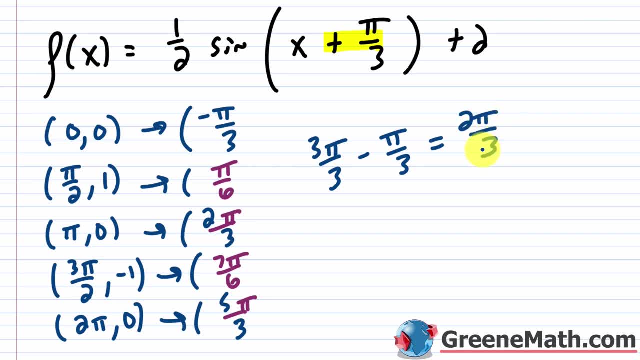 minus pi over three, And of course that gives you two pi over three. So you're getting the same thing. So it's the same result either way. You just have to be completely clear on which method you're using and what steps work with each method. I don't want anybody to get confused. 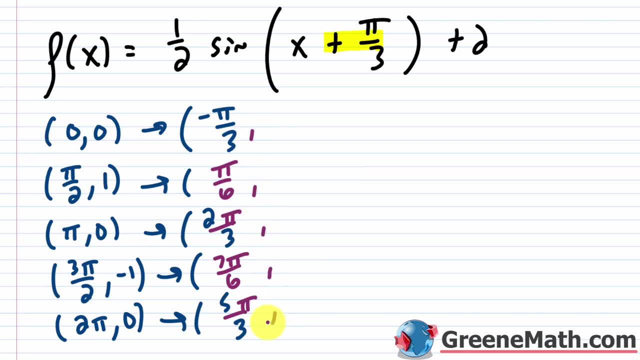 With that being said, let's go through and get our y values Again. you can always plug in, but you know that if you plug in negative pi over three right here, this part right here is going to become this right here. So if you plug in negative pi over three, you're going to get. 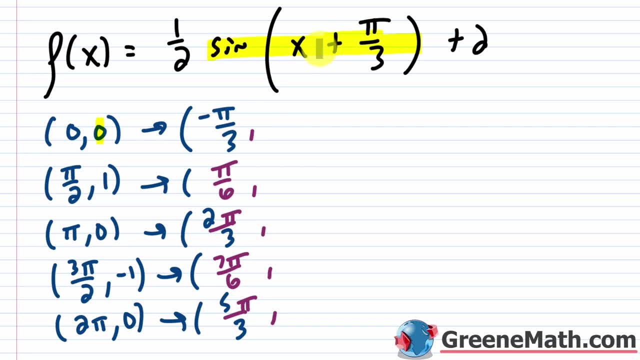 again negative: pi over three plus pi over three is zero. the sine of zero is zero. So this becomes this right here. So the shortcut is again just to use graphing transformations. you're just going to say: multiply by half times, whatever this is. So that's zero, then plus two. So then this would: 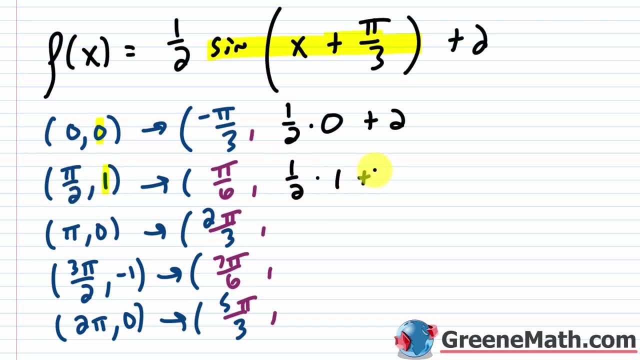 be one half times this guy right here, this one, and then plus two, so on and so forth. So this right here would be one half times your zero again, and then plus or two, And of course this is a duplicate of this. So you don't have to do this one. we can just erase this one. you could do. 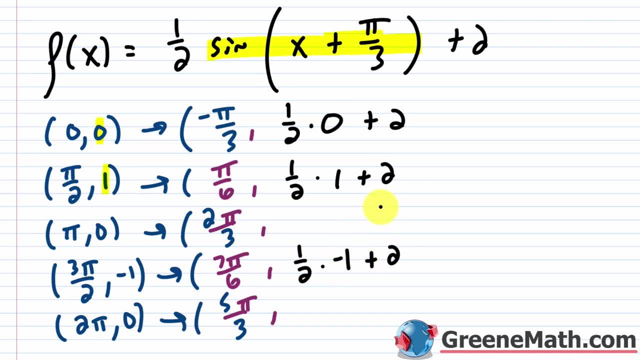 this one, So one half times your zero, and then plus two. So this would be one half times your zero and then plus two, So this would be two. we know that one half times zero is zero and you add two, so you get two. So this one's two, And of course this one's two, And of course this one's. 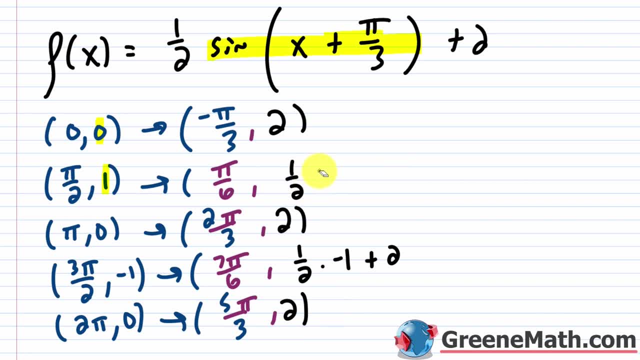 two For this. one one half times one is one half, and then plus two. you could say this is one half plus four over two, So this is five over two. So five halves is what you're looking for there. Okay, here this would be one half times negative one, that's negative one half, And then plus two. 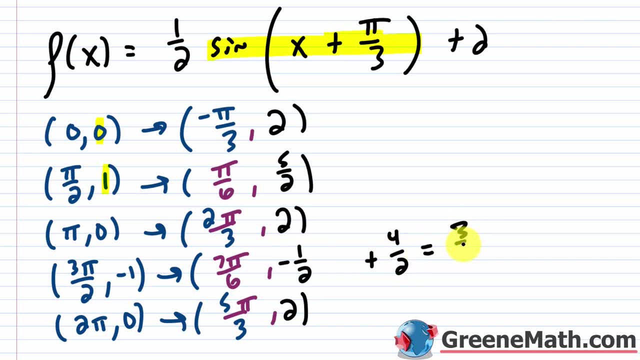 so let's say plus four over two And that would be three halves. so that would be for that one, So not too bad overall. Again, getting the Y values is always much easier. Let me go ahead and grab this real quick. 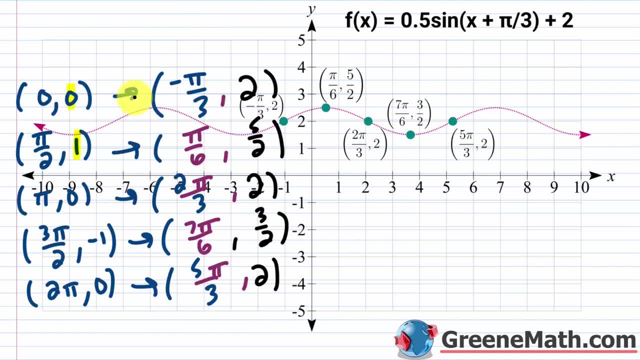 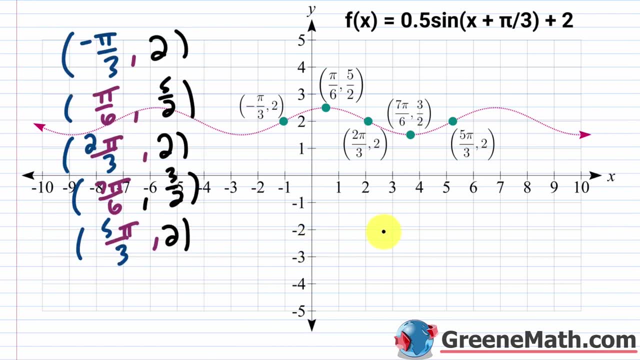 And let me come down here and paste this in: And really I don't need these, I just need these. So let me move this over so you can see everything Again. I gave you a link for Desmos, if you want to click on that. 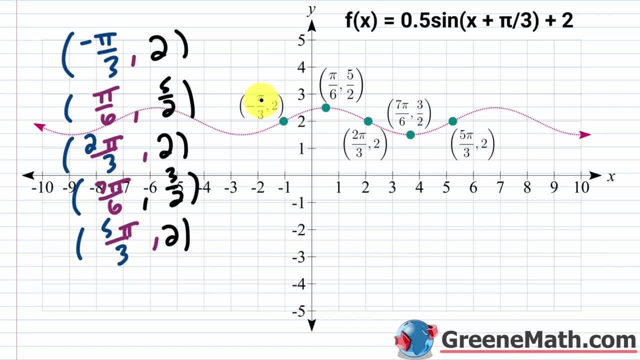 But essentially, when we graph this sine function as a guide, you have this negative pi over three comma two. you have this pi over six comma five halves. you have two pi over three comma two. you have seven pi over six comma three halves. 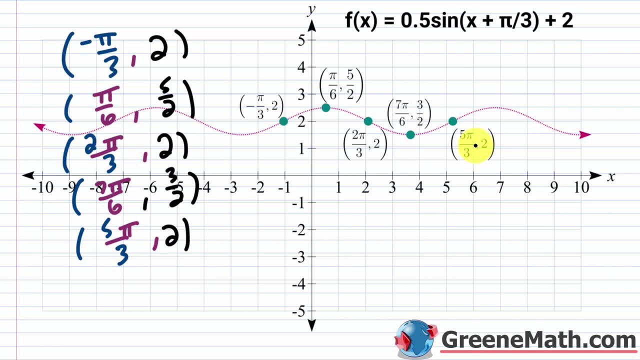 and then you have five pi over three comma two. Remember when you think about this at the beginning, the middle and the end. again, that's where you have your X intercepts on that basic sine function. This guy right here has been shifted up by two units. 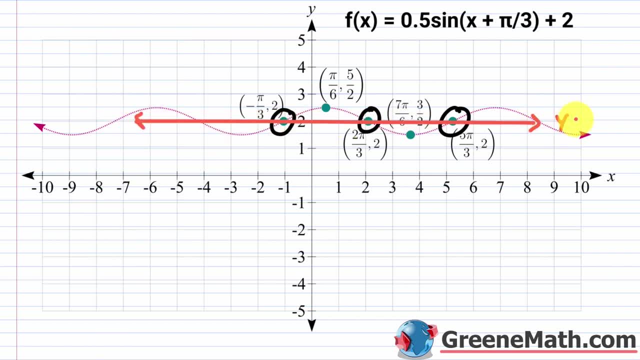 Again, this is what a lot of teachers do to make this crystal clear. So this is Y equals two. Again, it was Y equals zero, but you have this plus two here. that shifted everything up. So anywhere where you're hitting that line, Y equals two. 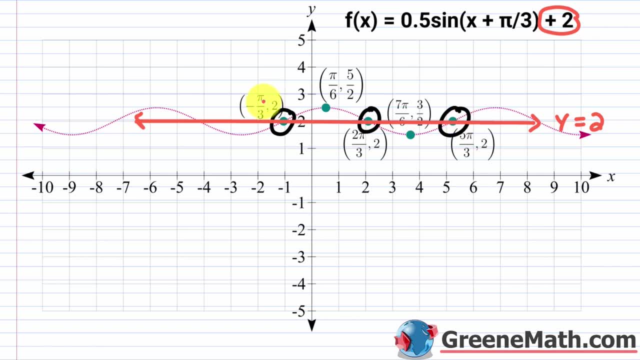 where your Y coordinate is two. so that means that the X value there that's going to be a place where the cosecant function is undefined, so you'd have a vertical asymptote. In other words, when I plugged in a negative pi over three, 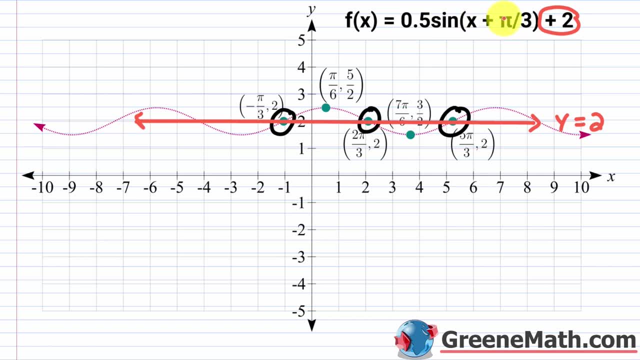 negative: pi over three plus pi over three, that's zero. the sine of zero is zero. But again, if you had the cosecant of zero, you would get undefined because the sine value is zero. Same thing would happen with two pi over three. 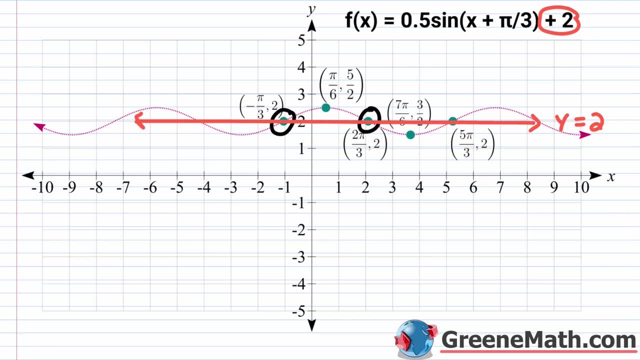 and this is five pi over three. Hard to see it because it's circled. Let me recircle it here in a smaller way. So the idea is you'd have a vertical asymptote: here at X equals negative pi over three, and then here at X equals two pi over three. 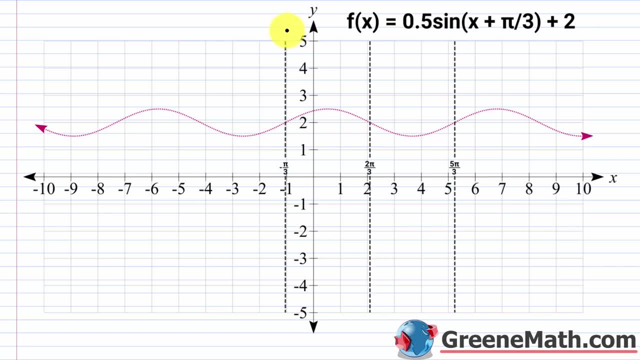 and then here at X equals five pi over three, So just showing this to you. So we draw these in as X equals negative pi over three, and then you can have X equals two pi over three, and then X equals five pi over three. 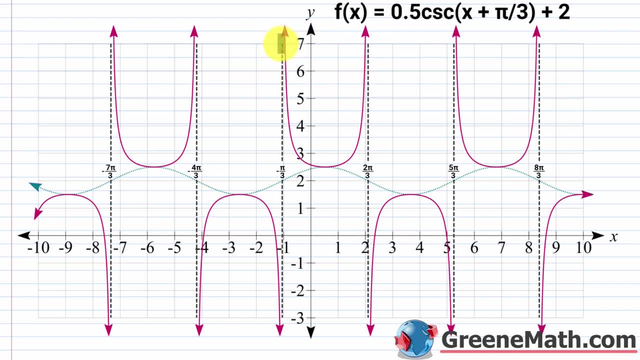 All right, so let's put everything together Again. here's your vertical asymptote: X equals negative pi over three. Here's your: X equals two pi over three. so another vertical asymptote. and then here's your: X equals five pi over three. 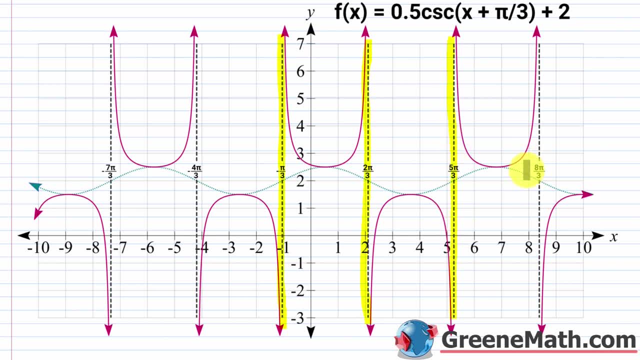 Of course, you can use your period to get additional vertical asymptotes going to the right or to the left, just depending on how far you wanna extend this. What I'm gonna do right now is just concentrate on what we worked on. So we know that we had a point that was. 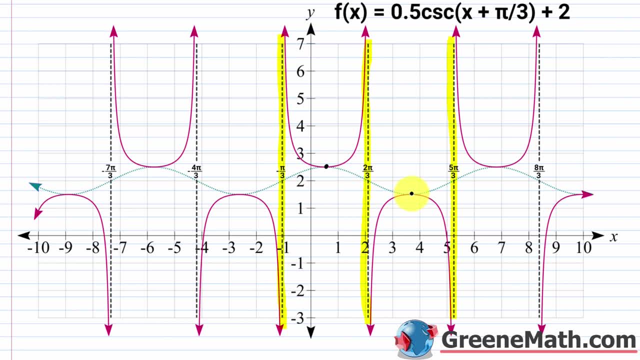 let's just say about right there. and then one that was about: let's just say: right there. So again you're going to interchange your hills and your valleys, So this right here is going to be a hill for the sine function, the guide function. 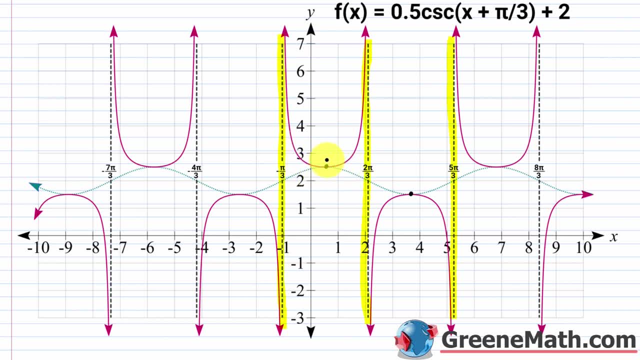 so that would mean that it's going to be a valley here. In other words, this maximum point on your sine function here becomes a local minimum on the cosecant function here, And then with this guy you have a valley on the sine function. 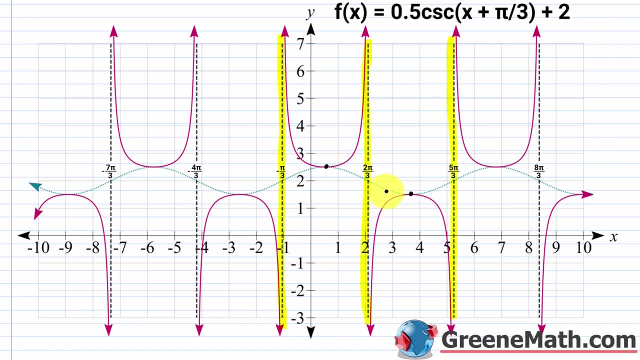 so that becomes a hill on the cosecant function. Or another way to say that is: you have a minimum on your sine function and then that's gonna turn into a local maximum on your cosecant function. So what we're gonna do is draw this. 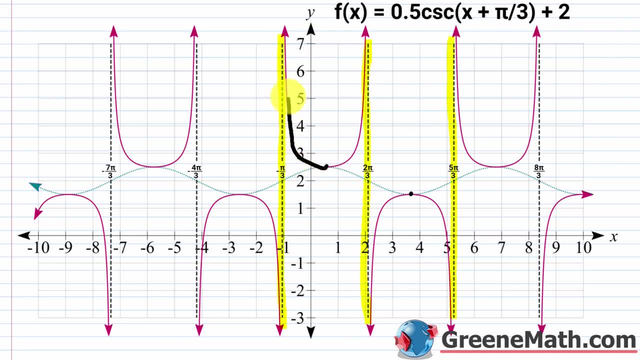 to where it approaches the vertical asymptote, but doesn't touch it. So there's that one, and then I'll do that over here as well, And then I'll come down here. same thing. So approaches the vertical asymptote, but doesn't touch it. 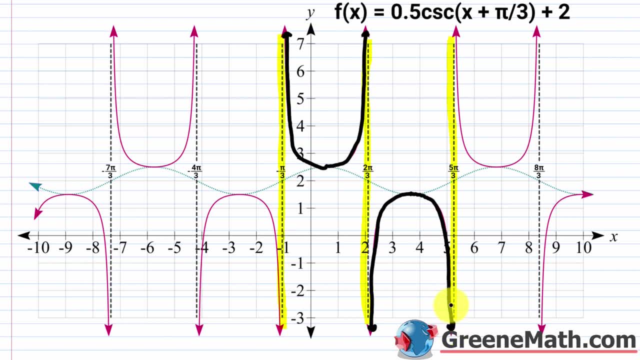 And then let me do this part right here. So again, that would be good enough for me. if I'm self-studying, you've done one period, So if you wanna continue this to the left or the right again, you have that link on Desmos. 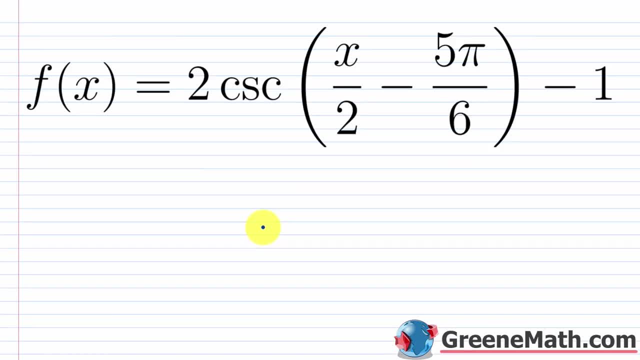 you can calculate all the things you need and then you could just use that link to check it. All right, let's take a look at another example here, with cosecant. So f of x equals two cosecant of x over two. 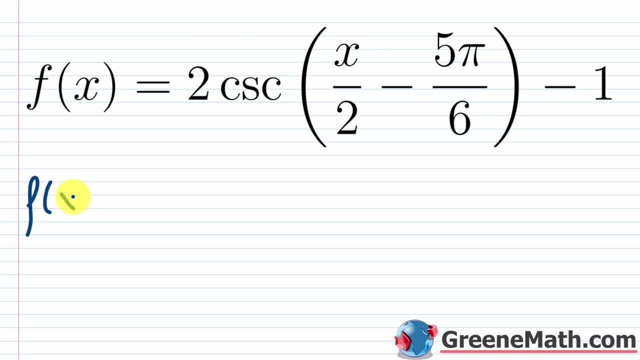 minus five, five or six and then minus one. So again I'm gonna factor this just to get things started. So f of x equals two cosecant of pull out a one half, And so inside you'd have x minus. 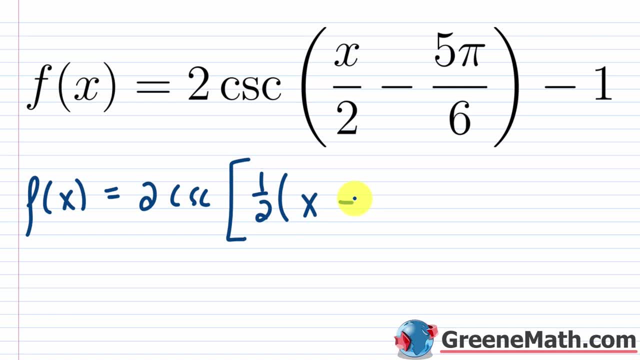 if I'm pulling out a one half, how do I undo multiplication by half? I need to multiply by two, So this one you might need to write it out. So five pi over six times two, And so this would cancel with this. 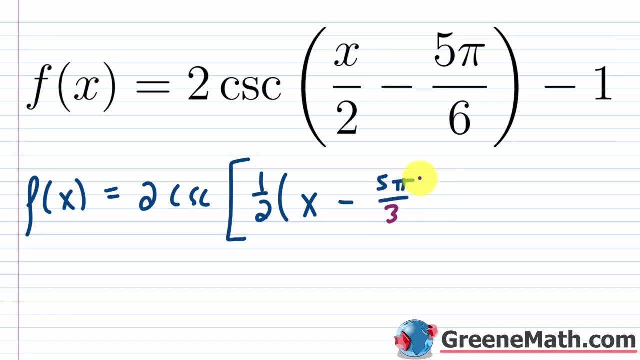 and give me a three down there. So this is five pi over three And I know this gets a little bit tricky when you're factoring like that, but you can always check it. A half times x is one, half x or x over two. 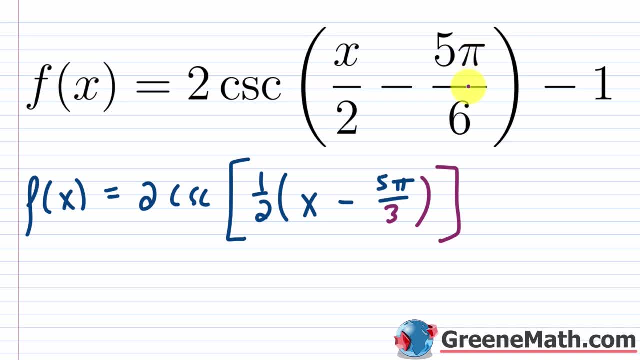 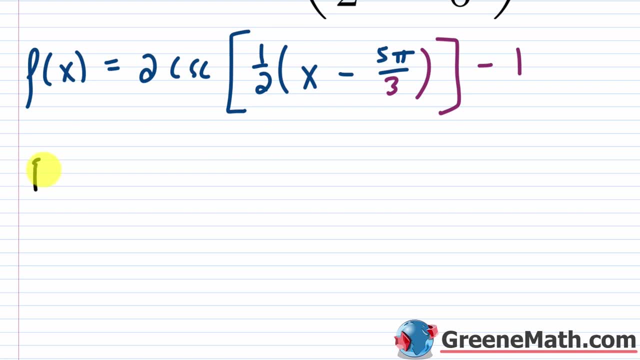 Then minus and minus one half times five pi over three, that is five pi over six. So that checks. So then we have minus one. So at this point we can just get the phase shift right away. That's why I factor. 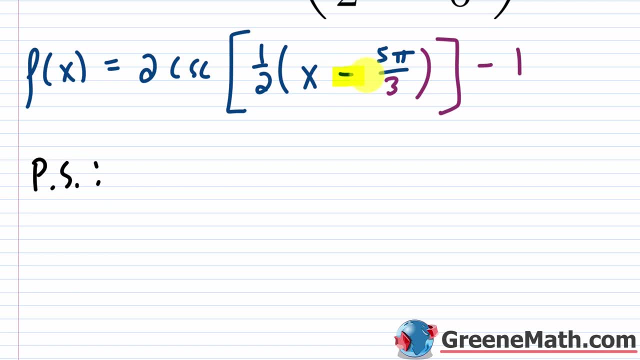 So for the phase shift you're gonna get again. how do I undo this minus five pi over three? I need to add five pi over three. So I'm going to the right: five pi over three. This part right here is a vertical shift. 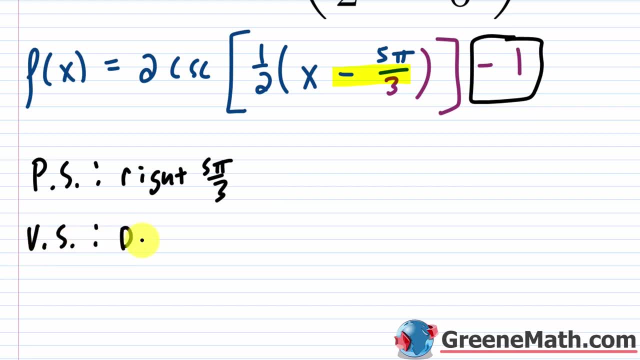 going down by one unit. So vertical shift, So it's down one unit Then for the period. so for the period you look at this one half here. that again is the coefficient of x in unfactored form. In factored form it's outside the parentheses. 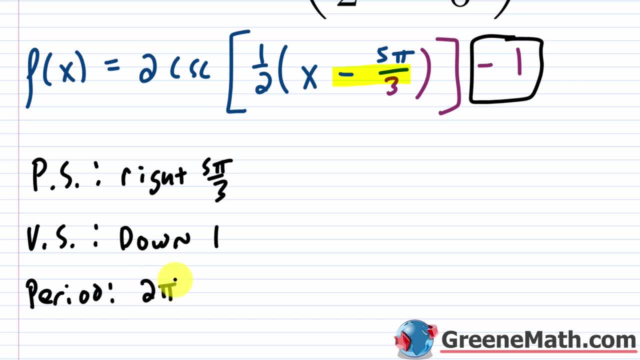 but essentially you take your two pi, which is your standard period, and you divide by a half. Well, if I divide by a half, it's like multiplying by two. So this gives me four pi for the period, If you want the quarter period. 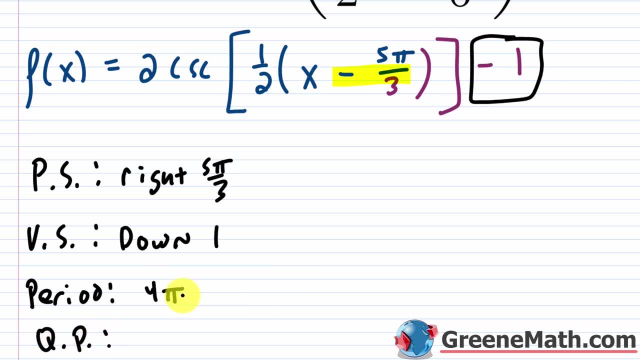 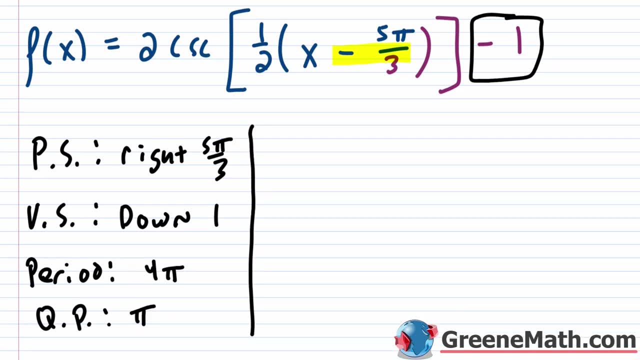 because you're using that method. so the quarter period, well, you just take four pi, you divide by four, you get pi. That's all it is. If you want to do graphing transformations, again, it was more simple on the last one. 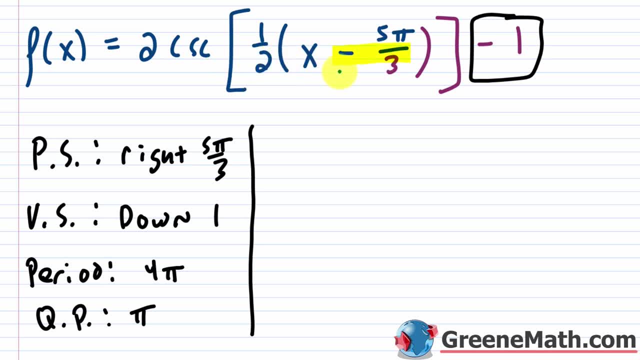 This one. you have two things that are happening on the inside. So again you've got to undo things, and to undo something you have to go on the reverse order. Essentially, if you look at this, I'm going to go inside of the parentheses first. 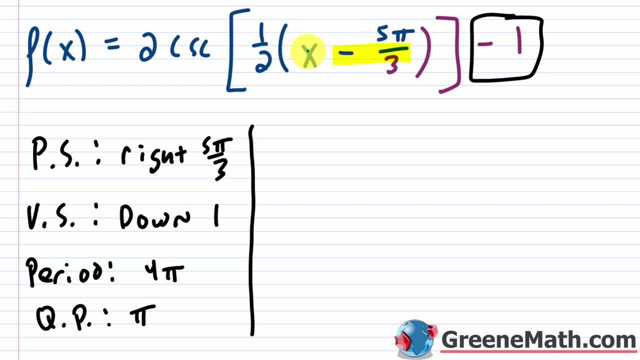 if I'm using the order of operations. I know you can distribute this, but just the way it is, I would go inside of this first and then I would multiply second. So I've got to undo this in the reverse order. So now this is one and this is two. 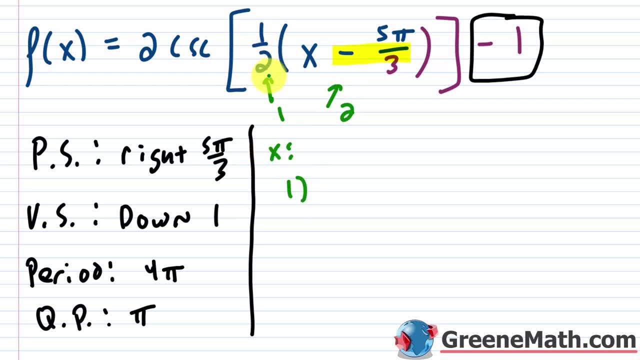 and I'm undoing things. So, for x, how do I undo multiplication by a half or division by two? Well, I'm going to multiply by two, So I'm going to multiply by two. So, in other words, I have a horizontal stretch by a factor of two. 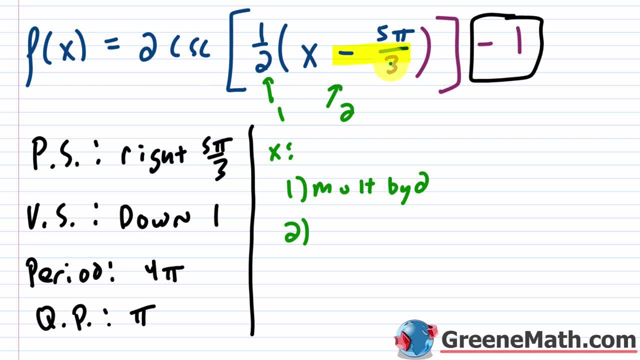 Then this guy right here: I need to undo the subtraction of five pi over three. Well, that means I need to add five pi over three. So I'm going to add five pi over three and that's shifting me to the right by five pi over three. 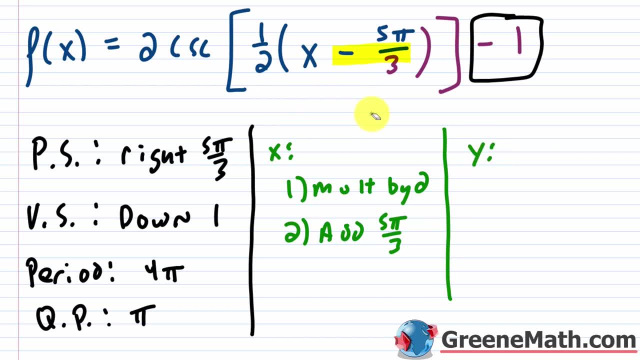 Then again for the y. this is always much easier and very straightforward. You just follow the order of operations. So you have that two. that's multiplying this, So we're going to multiply by two and that's going to give me a vertical stretch. 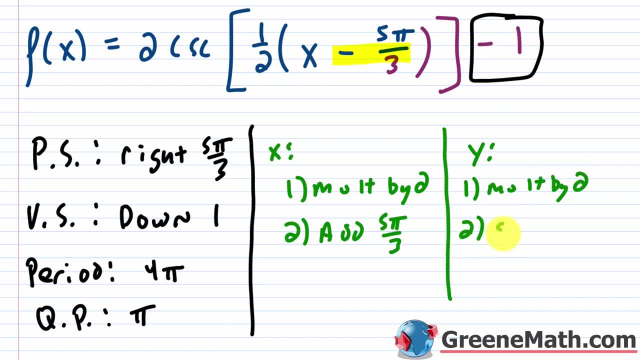 by a factor of two, And then the second thing is you have this minus one, So we're going to subtract one, and then that is just going to shift me down by one unit. So if you want to use this, that's fine. 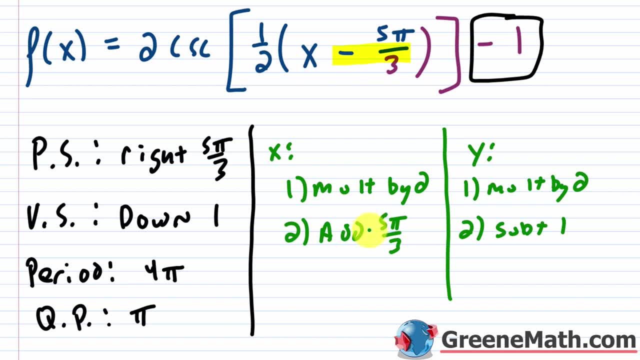 You just take those original points for your sine graph and then you take the x coordinates. You're going to take each one, multiply by two and then add five pi over three. That's going to be slower in this case because of getting common denominators. 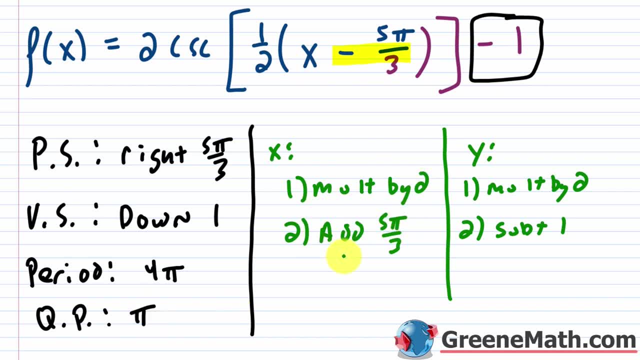 It's going to be faster to use the quarter period method, So I'm just going to stick with that. Maybe I'll show you one or two points with this, just for clarity. So let me go ahead and grab this and let's paste this in. 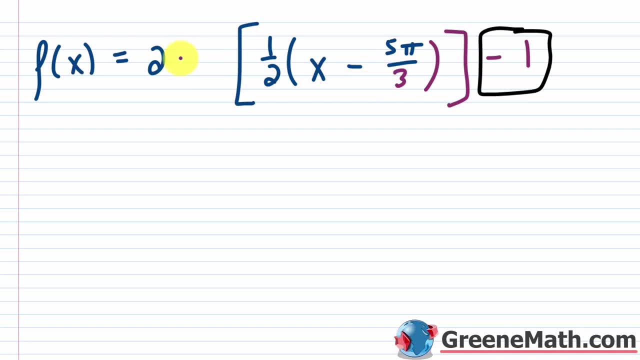 And of course, what we're going to do is get rid of that cosecant And we're going to sketch the graph of the guide function. So we're going to put in a sine and make the n better there. All right. so once we look at this, 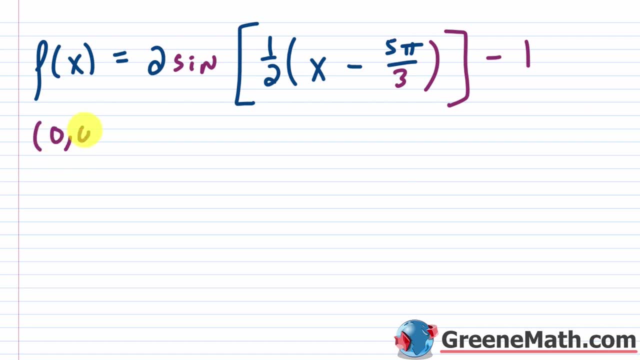 again you think about your basic points for the sine graph. So you have zero comma zero. You have pi over two comma positive one. You have pi comma zero. You have three pi over two comma negative one, And then you're going to have two pi comma zero. 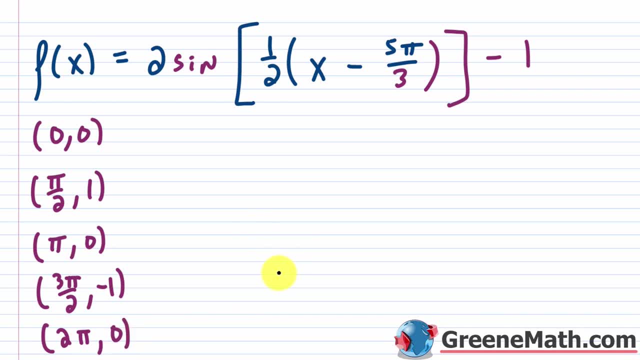 All right, so let me start out by doing the quarter period method And then, once we've done that, I'll do a few points using the graphing transformations. So the quarter period here is going to be pi. Now your phase shift is plus five pi over three. 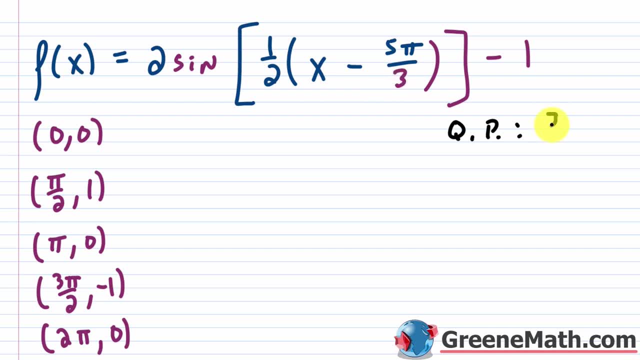 So what you'd want to do is write this with a common denominator And you could say: this is three pi over three. That three could be a lot better, And so the first thing here is going to be: I'm just going to shift to the right by five pi over three. 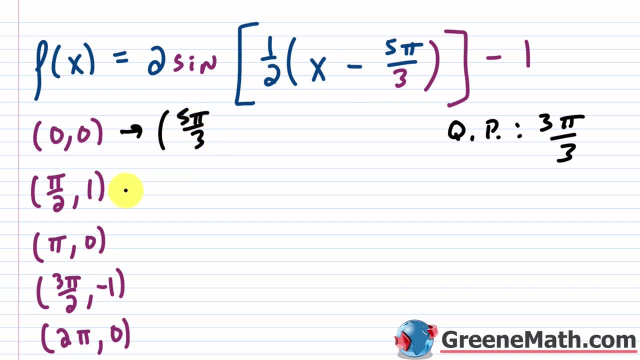 So I'm going to say, instead of zero, now I have five pi over three, And then to get the additional guide, I'm going to do this. So instead of adding pi's here, you're just going to keep adding quarter periods. 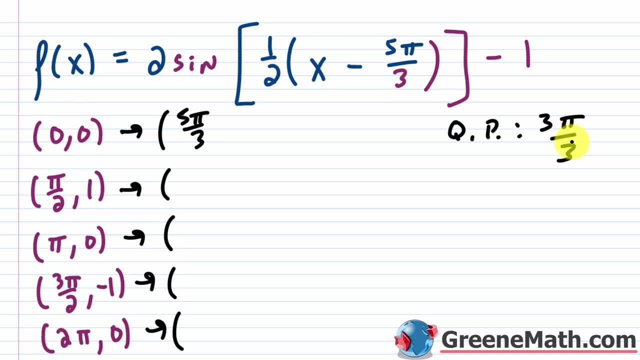 So don't worry about these x values here, You're done with that. You just want to add this guy right here to this guy right here and then just keep going. So five pi over three plus three pi over three, that is eight pi over three. 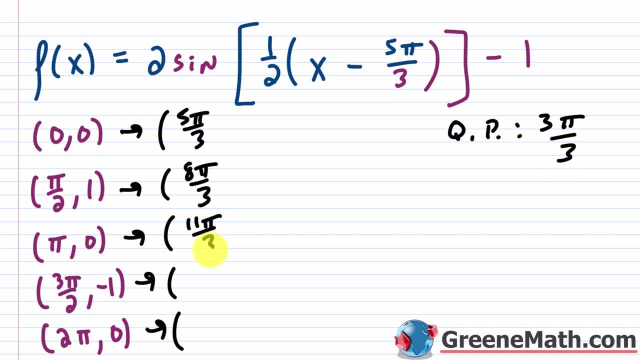 Then eight pi over three plus three pi over three, that is 11 pi over three. Then 11 pi over three plus three pi over three, that is 14 pi over three. That one could be better. And then 14 pi over three plus three pi over three. 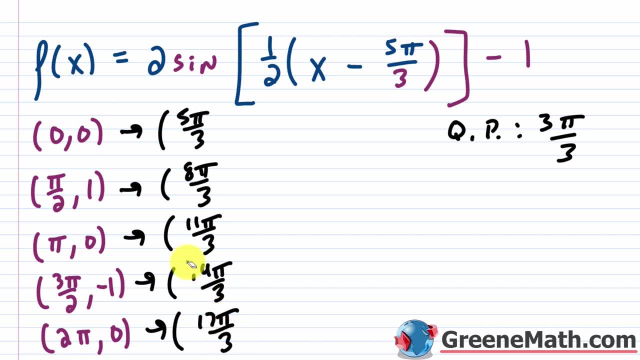 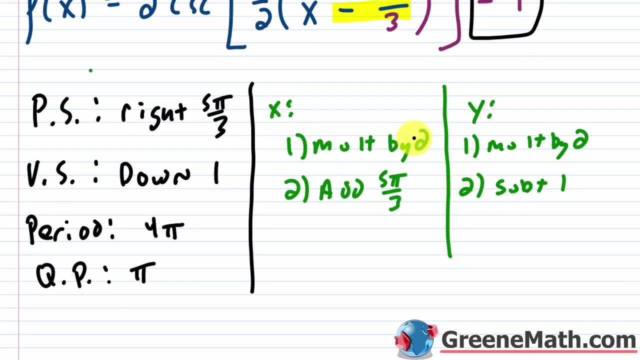 that is 17 pi over three, So it's pretty quick in a lot of cases. once you get a common denominator, All right. so the next thing is: if you wanted to try this with graphing transformations, again, we were told to multiply by two. 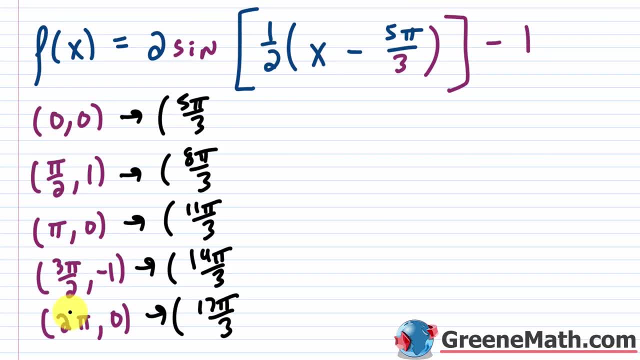 and then add five pi over three. So with this one you are working with these x values. This one you can just skip because you're multiplying by zero first and then you're adding five pi over three, So of course you're going to get five pi over three. 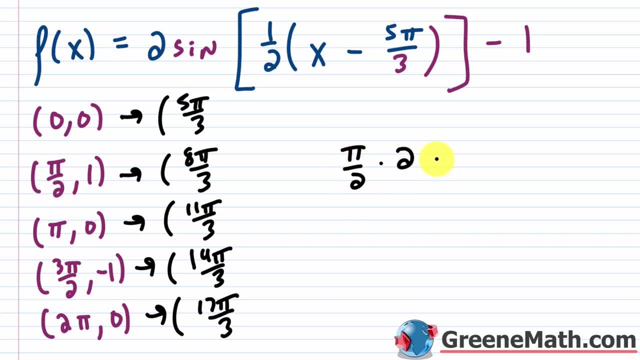 But for this one let's just try it. So pi over two, you're going to multiply by two first and then add five. pi over three. So let's say, if we do get eight pi over three, So this right here, we cancel. 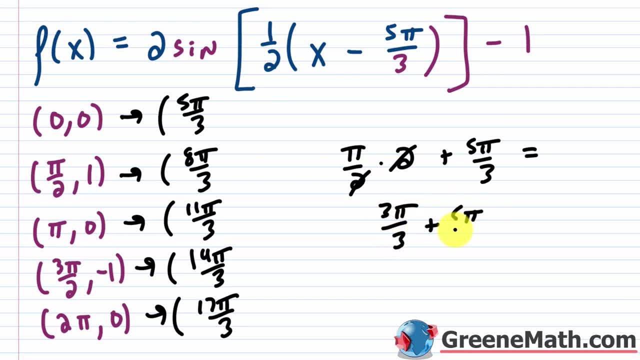 And what do you get? You get three pi over three plus five pi over three- Let me make this five better- And of course you do get eight pi over three. So let me get rid of this And you can see that works. 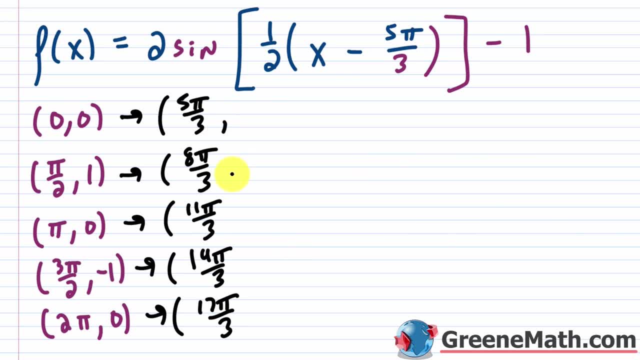 If you want to do the rest of them that way, that's up to you, All right. so for the other guy we need our y coordinate, And for that we're going to use graphing transformations. Again, if you plugged in five pi over three. 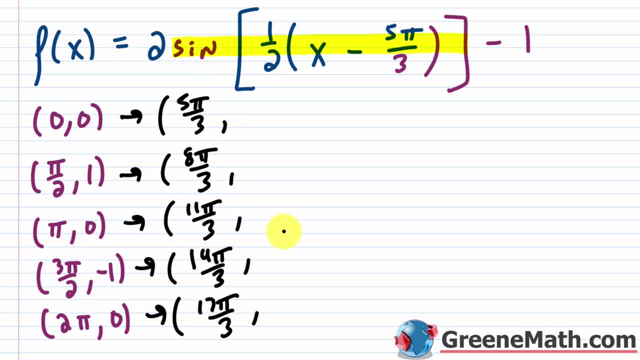 this part right here would turn into zero. So to shortcut that, all you have to do is say: well, I have this guy two right here times. whatever this would be, In this case, it would be zero, And then you have minus one. 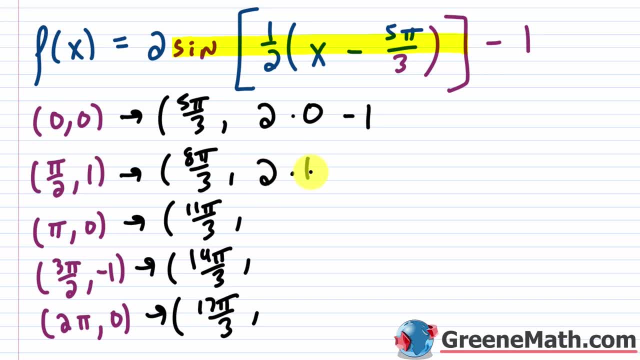 And then for this one it would be two times. this would be one and then minus one, And this is going to be a repeat, So we just have to do this one, So you would have two times Again. this, right here, would end up being negative one. 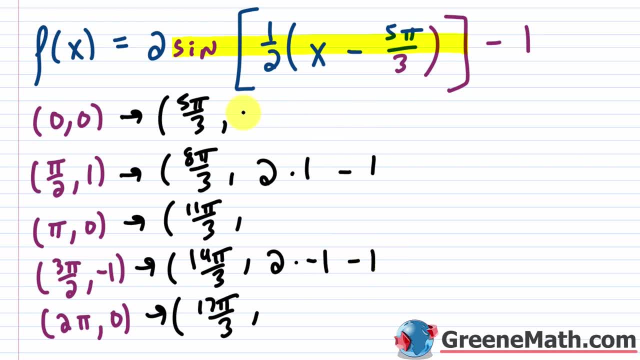 and then minus one. So two times zero is zero. And then you have minus one, which is just negative one. So minus one two times one is two. Minus one is one. So you can put that there, And then this one's just going to be a copy. 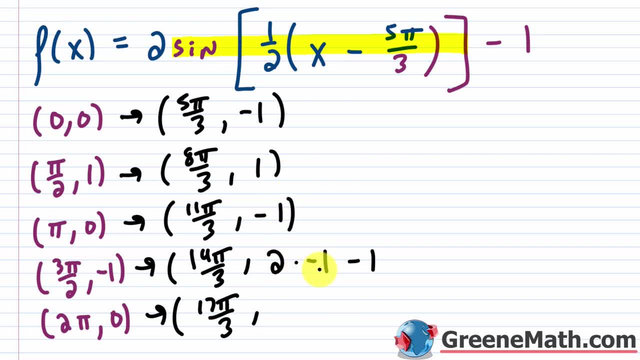 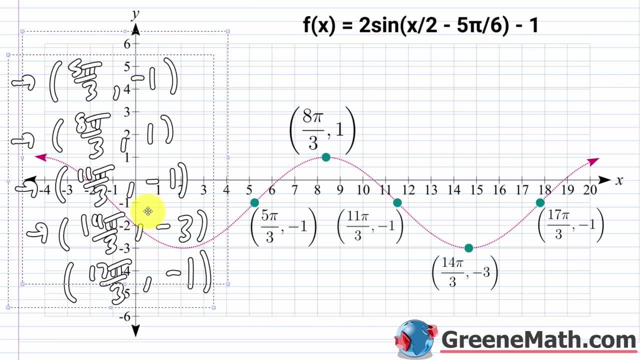 So it's negative one, And then two times negative. one is negative two. Negative two minus one is negative three. So this is negative three And then this one you can copy. it's negative one. Okay, let me paste this in here real quick. 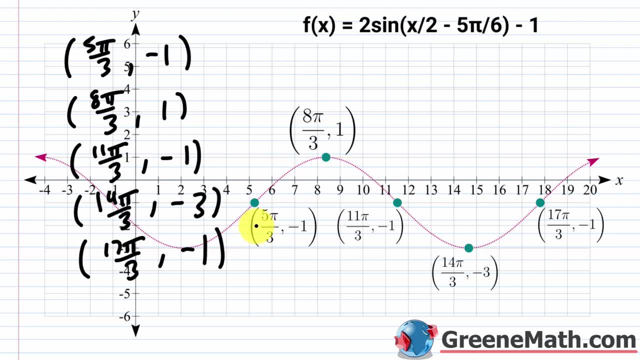 I'm just going to erase this. And so at the beginning of the cycle you have five pi over three comma negative one. Then at a quarter of the way through you have eight pi over three comma one. Then at the middle part. 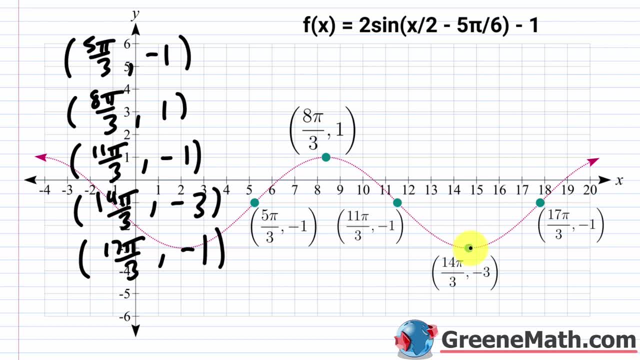 you have 11 pi over three comma negative one, Then, three quarters of the way, you have 14 pi over three comma negative three, And then, finishing up the cycle, at the end, we have 17 pi over three comma negative one. So you can get rid of these. 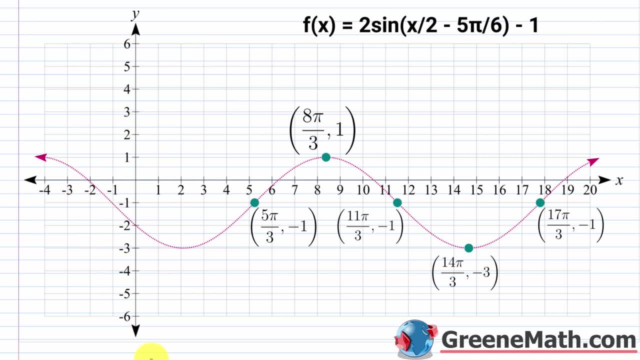 Again where you're looking for where to put your vertical asymptotes again at the beginning, the middle and the end. So just remember that beginning, middle and end, The horizontal line that passes through the middle of this guy is going to be at y equals negative one. now, 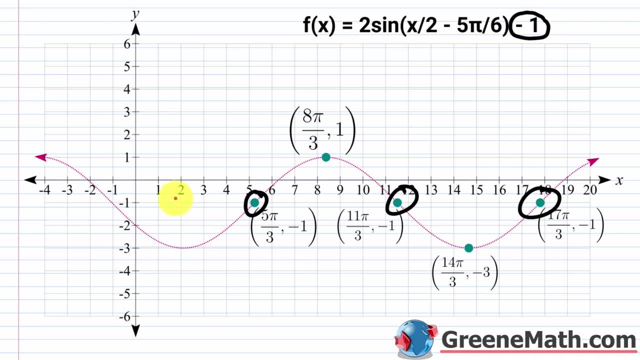 because you've shifted down by one unit, You have that minus one there. So this is y equals negative one there. A lot of teachers do this to say, hey, if you have a point that hits that midline there, well, you want to take the x value there. 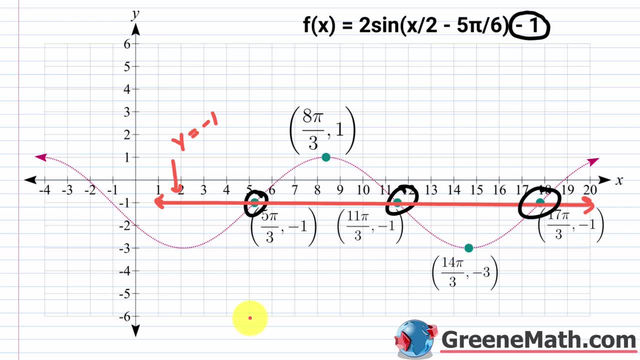 and you're going to use that to create a vertical asymptote for your cosecant function. That's all you have to remember. So we'll have one at five pi over three, 11 pi over three and then 17 pi over three. 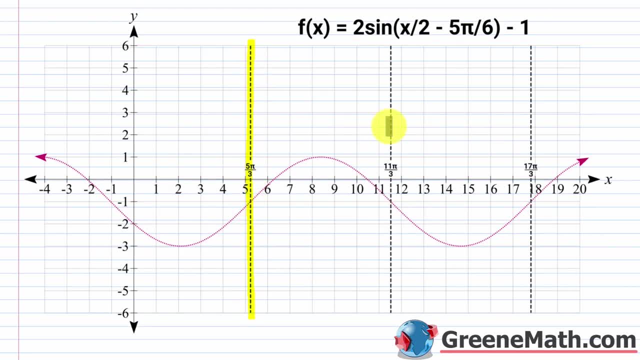 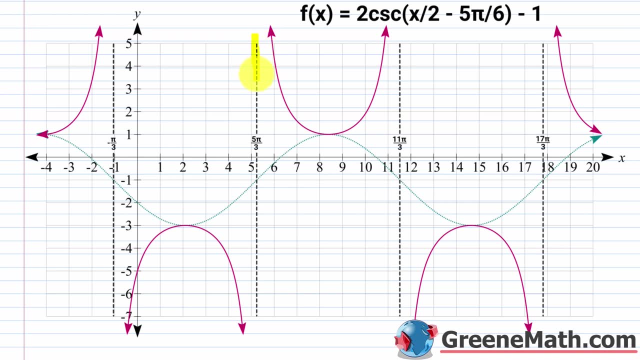 So there's your vertical asymptotes. Again, here's one at five pi over three, here's one at 11 pi over three, and then here's one at 17 pi over three. So putting everything together, let's do again: the x equals five pi over three. 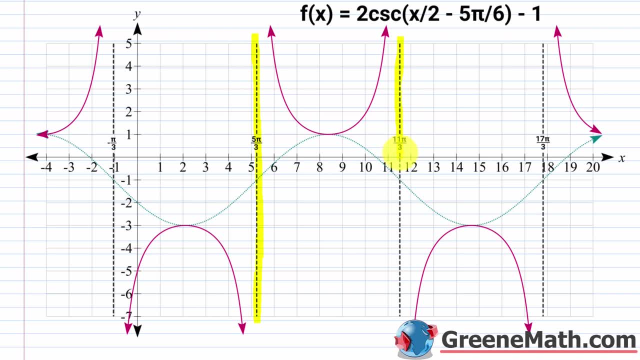 a vertical asymptote. And then the other one that we saw: x equals 11 pi over three. And then the last one that we found was x equals 17 pi over three. So we've got those Again. you can always get ones to the left or the right. 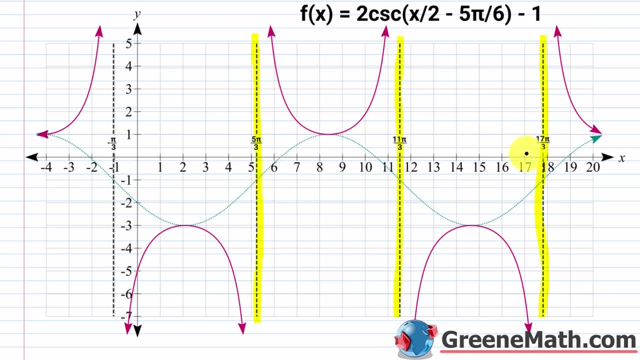 going as far out as you want. And then in this cycle here we know that we found a point. let's just say it's about right there. And we had a point again. let's just say that one was about right there. 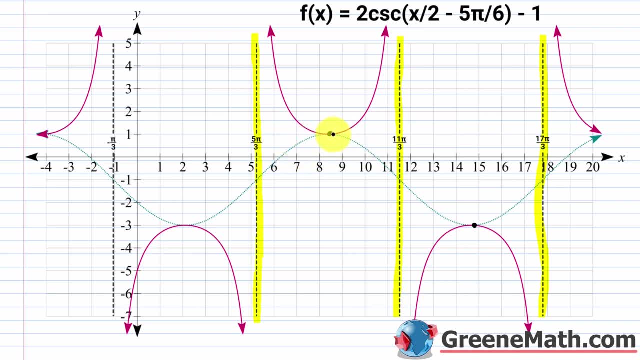 So the idea here is that this hill on your sine graph- the guide graph, is going to become a valley on the cosecant graph, Where, again, you can always say that this maximum here on the sine graph will turn into a local minimum here. 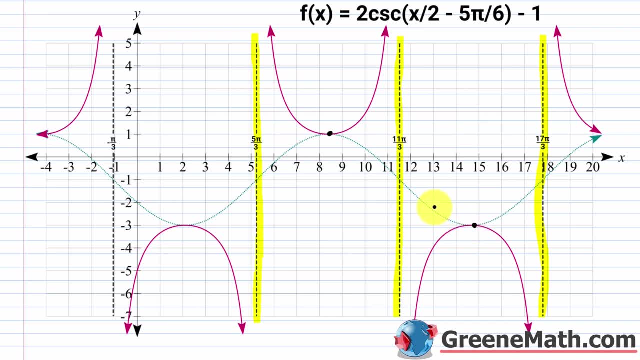 on the cosecant graph. Then, when we get to this point, here again this is a valley on the sine graph, so it becomes a hill on the cosecant graph. Where again, another way to say that is that this minimum here on your sine graph. 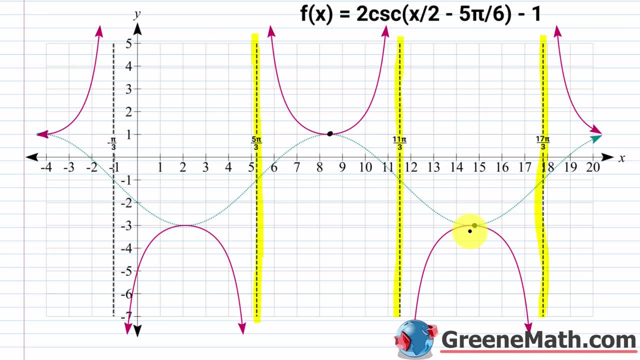 is going to become a local maximum on the cosecant graph. So once you have that down, you're just going to sketch this guy again to where this is going to approach the vertical asymptote, but not touch it. And again, just approach the vertical asymptote. 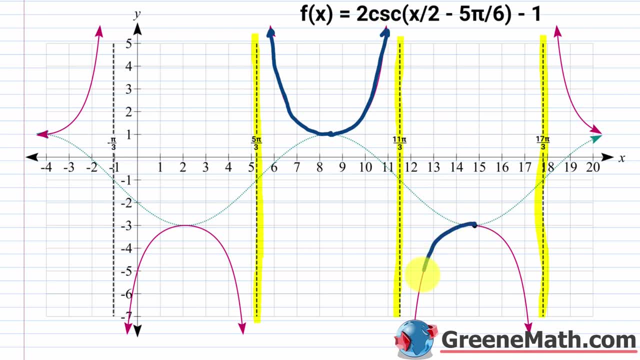 and not touch it. And then this guy will do the same thing, the same thing here. So approach the vertical asymptote and not touch it. and then approach the vertical asymptote and not touch it. Once again, I gave you a link on Desmos. 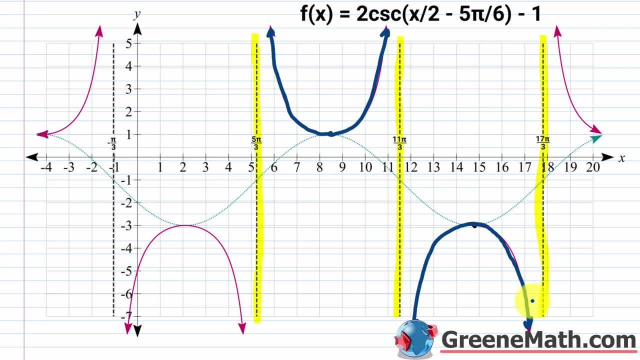 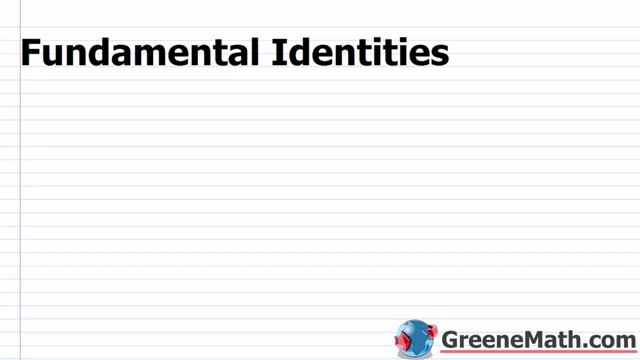 If you want to do some additional practice, you can go to the left or to the right by as much as you want and just use Desmos to check your work. In this lesson we want to talk about fundamental identities in trigonometry. 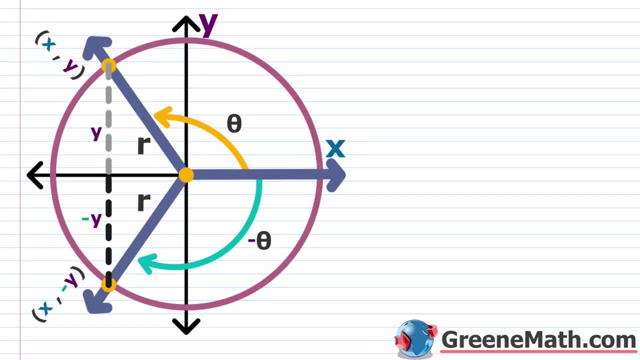 So at this point, we've already talked about the reciprocal identities. We've talked about the quotient identities and the Pythagorean identities. If you forgot all that stuff, because it's been a while since we covered it, it's okay. I'm going to pull up a quick little cheat sheet in a moment. 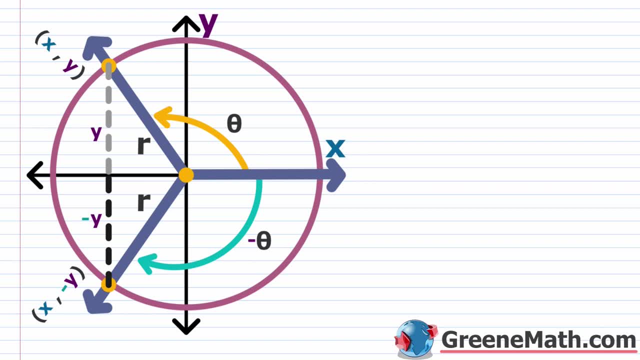 Before we get into what we can do with the fundamental identities, I've got to give you one other piece of this puzzle. okay, And that's going to be the negative angle identities which some books call the even odd identities. okay, So it just depends on your textbook. 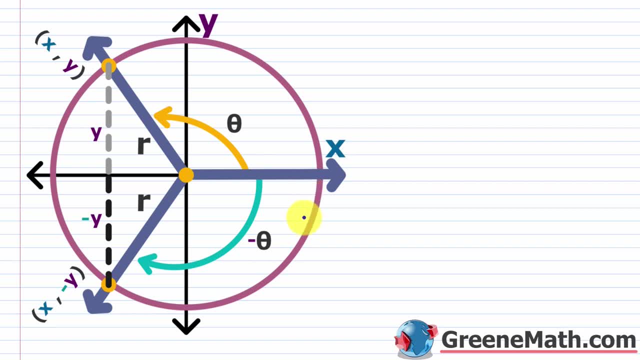 which name you're going to use. Now, when we look at this little graph here, we're going to consider two angles. One is going to be this angle: theta. okay, So here's your initial side, here's your terminal side. 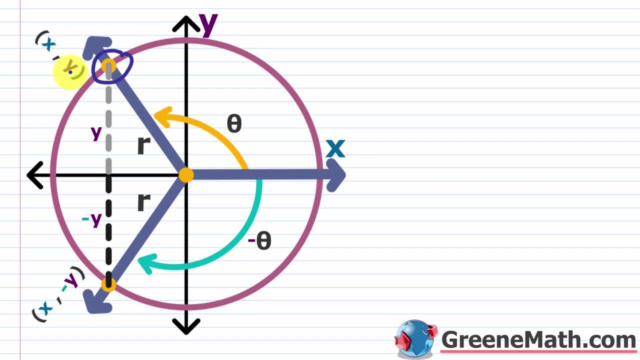 And you can see, this point here on the terminal side is just marked with X comma Y, just generically. If I had a negative theta, so the negative of this guy. so now we're moving clockwise. Well, this point here on the terminal side. 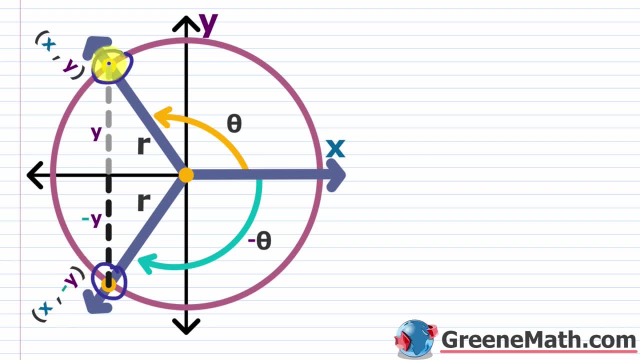 notice how it's X comma, negative, Y right. So this is the Y up here and this Y down here is the negative of that. Notice how the X value is the same. okay, So we're going to use that to build this little relationship here. 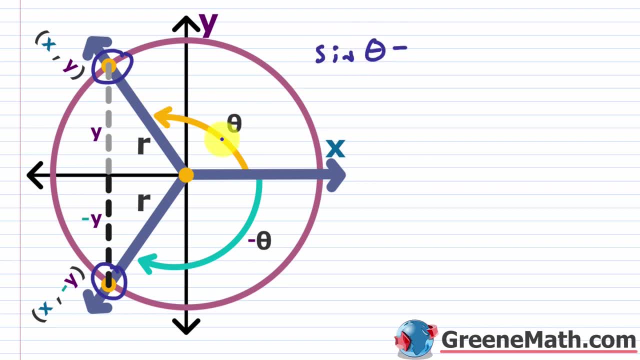 We're going to first start with sine of theta. okay, So sine of this guy right here, this would be equal to what It's always Y over R. But when I think about sine of negative theta now, how do things change? 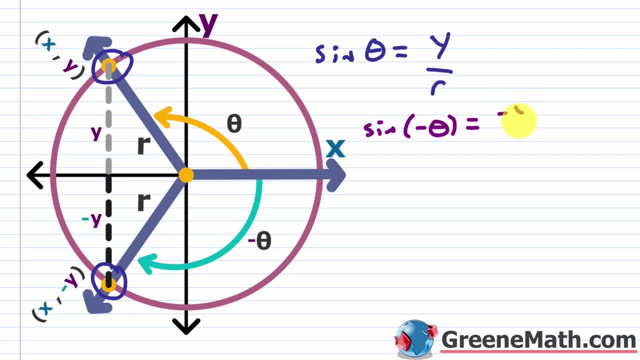 Remember, now I'm dealing with the negative of Y okay. So the negative of Y over it's still going to be R, okay. So what I can see here is that these guys are going to be negatives of each other. This guy is Y over R. 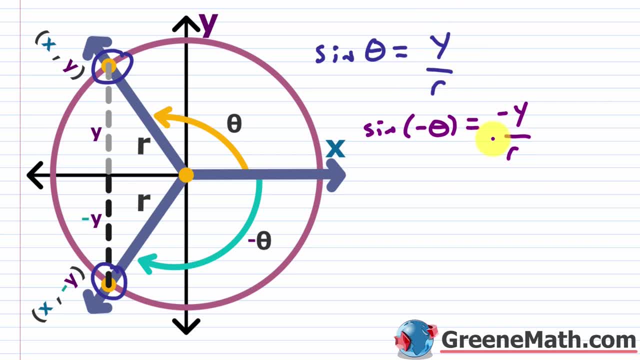 and this guy is going to be the negative of Y over R, So I can use that to build a little relationship. that's always going to be true, And I can just say that the sine of a negative theta is always going to be equal to. 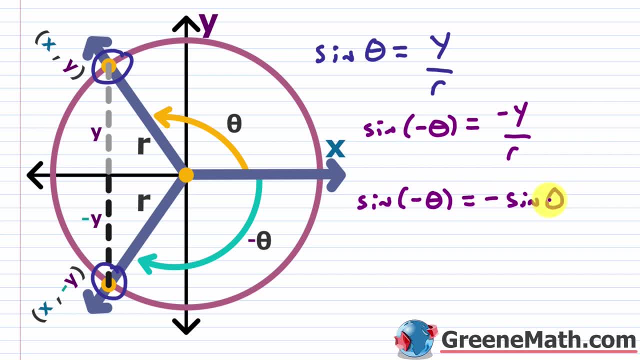 the negative of the sine of theta. okay, So this is your first negative angle identity. Now you might notice that this looks very familiar from earlier, when we worked with functions and we talked about even and odd functions, right. This property here is from odd functions, right. 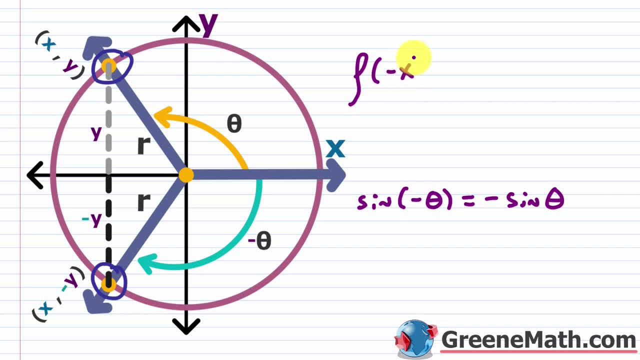 So this is an odd function. If you had something like F of negative X and you said this was equal to R, okay, to the negative of f of x, remember, this is an odd function. that's how you check for it, so let's. 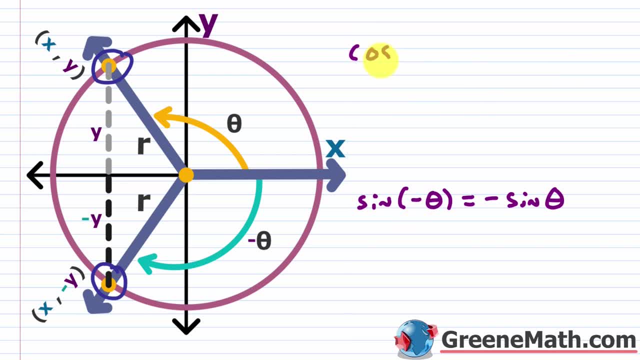 erase this and think about cosine now. so with the cosine of, let's say, theta, okay, what is it? it's x over r, so it's x over r. but now when i look at the cosine of negative theta, okay, it's the same x. right, the x is the same. you have x comma y, you have x comma negative y, so x is not changing, okay. 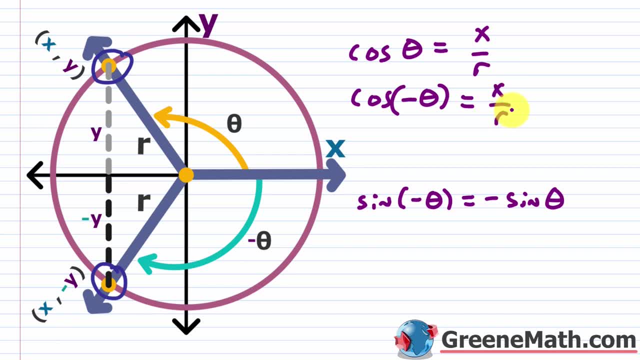 so we can say that the cosine of theta is equal to the cosine of negative theta. remember, this is a property of even functions. so we'll say that the cosine of theta is equal to cosine of negative theta. okay, all right. so, lastly, i'm going to take the relationships here and i'm going to build. 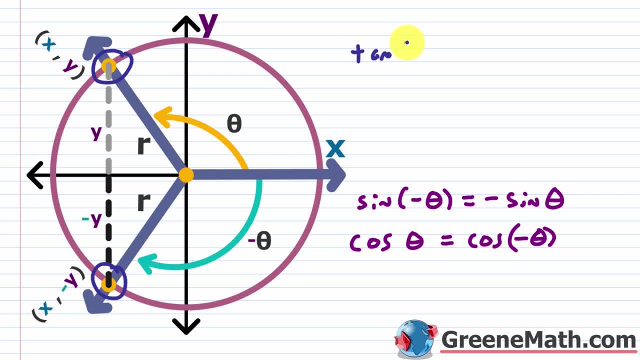 something with tangent. okay, so i know that the tangent of theta is equal to the sine of theta over the cosine of theta. now let's think about this: if i had a negative theta, then all of these would just be negative theta, right? so if i erase this and put a negative theta 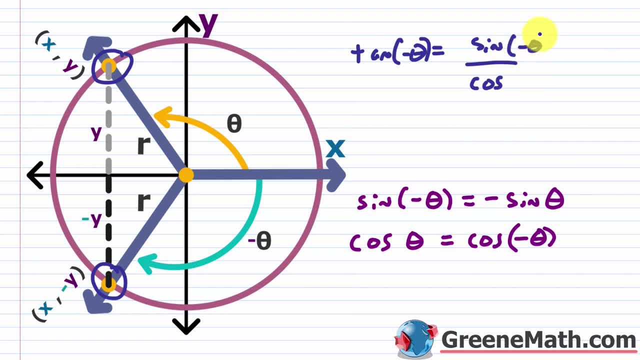 and i erase this and this and i just put a negative theta in here and a negative theta in here. what i want to do is think about how can i take what i just found here, plug it in there and simplify and come up with something? well, basically, we know that the cosine 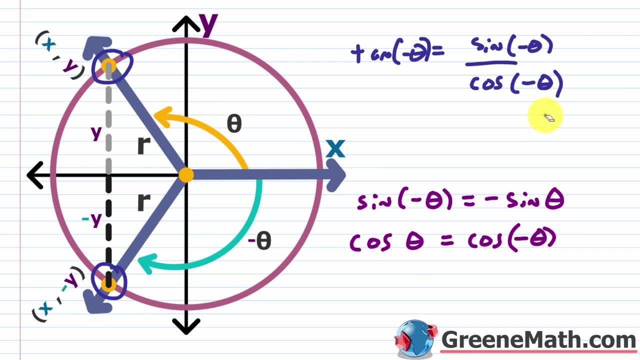 of negative theta right here, tells me that's the same as the cosine of theta. so i can erase this and go back to the cosine of theta. and i can take this guy right here: the sine of negative theta. and i can take this guy right here: the sine of negative theta. and i can take this guy right here. 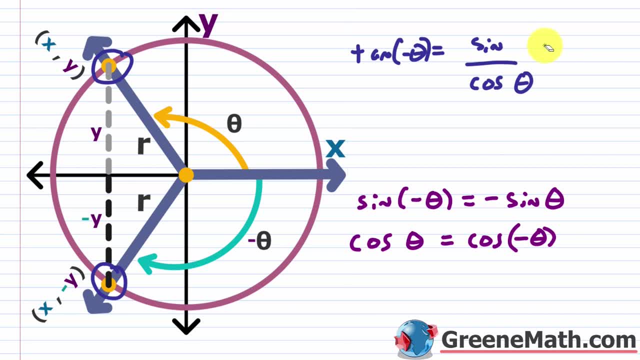 and i can basically pull the negative out in front. so let's get rid of that, okay, and i'll pull that out in front. so what does this tell me, if i compare this one to the one i just had? so the tangent of theta, where it's the sine of theta over the cosine of theta, where they're negatives of. 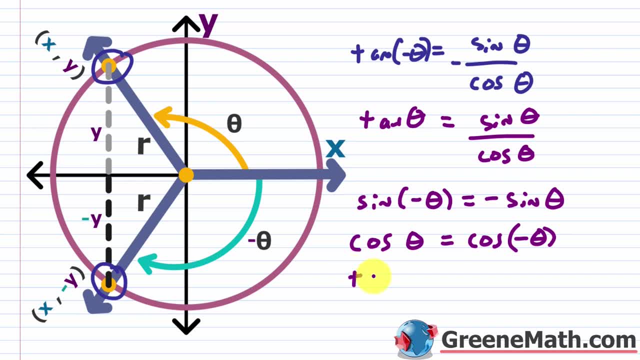 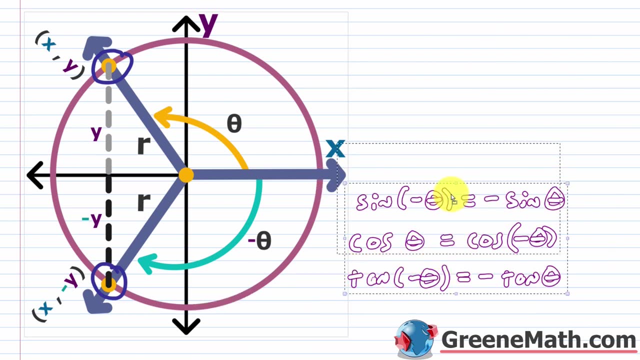 each other, right? so just like this first relationship, so we can say that the tangent of negative theta is equal to the negative of the tangent of theta. all right, so let me erase this. i don't know what that's asking me here. yeah, negative theta is 0 to the Poisson tragedies. 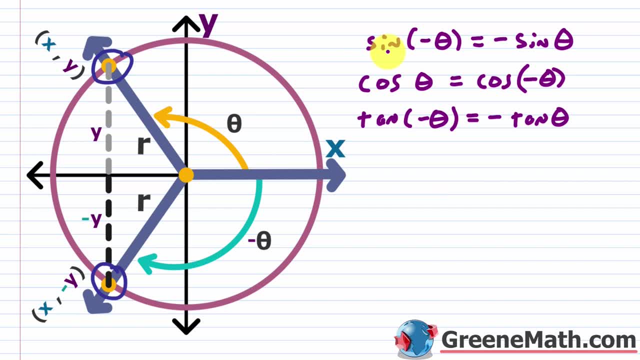 okay. so what does that say? okay? so it says, yes, the the maximal moments are equal to the exponential moments. okay, so when you take the of theta low, if you can read this, then that means you know you're in the right place. with uh, what does that say? yes, timeяться. just saying if that. 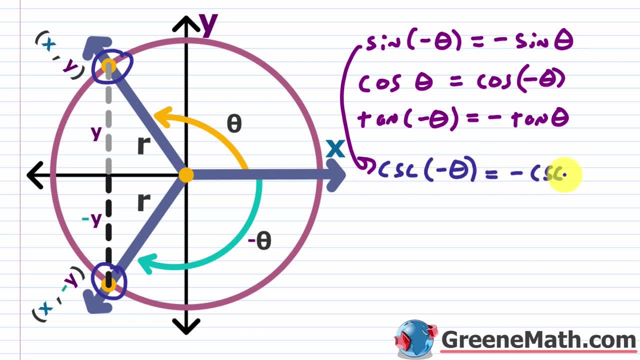 was the obsessed graduate didn't mean we don't have time to compute these number of milliseconds, right. we can just take this one out at the right time with the angular moments. okay, and we can use reciprocal. that's going to be secant, right, so i can do here. i'll drag this down here. let me change. 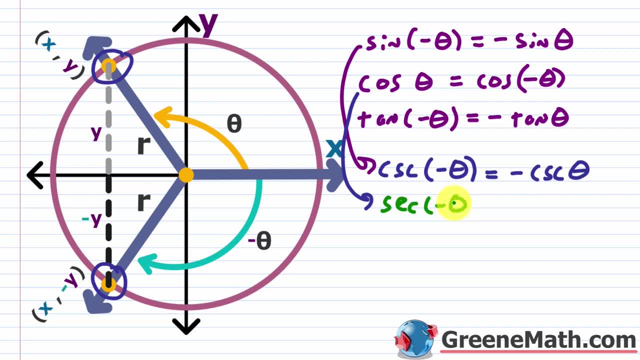 my color. the secant of, let's say, negative theta will be equal to the secant of theta. okay, so those match. then lastly, this guy right here: let me change the color one more time. i think i'm running out of ink, so let me use this one. so here with the tangent. again, it's going to be if you flip it. 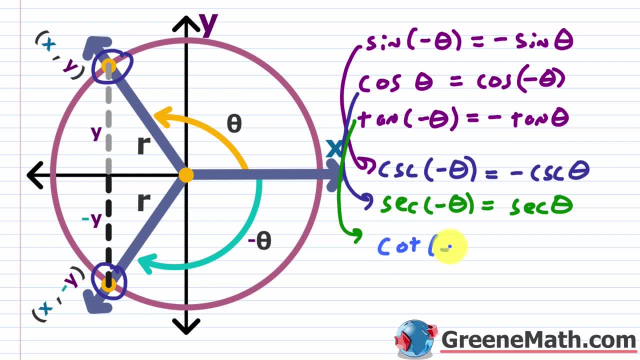 you get cotangent, so i'm going to say that the cotangent of negative theta is equal to the negative of the cotangent of theta. okay, so these are the negative angle identities, or some books again call it the even odd identities because of when we're talking about even and odd functions. 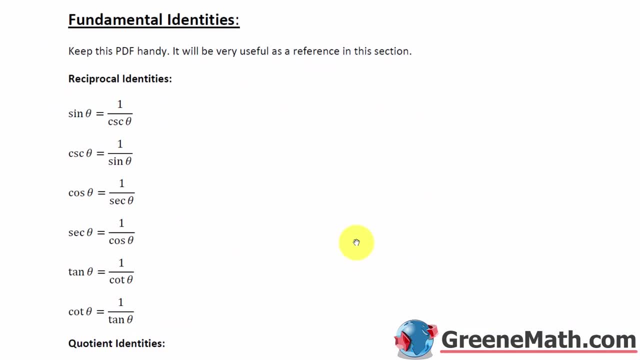 now i want to pull up this little pdf which is attached at the beginning of this section for you, okay. so i say, keep this pdf handy. it's going to be very useful as a reference in this section. you want to start by just going back and forth and reading things and writing it out. 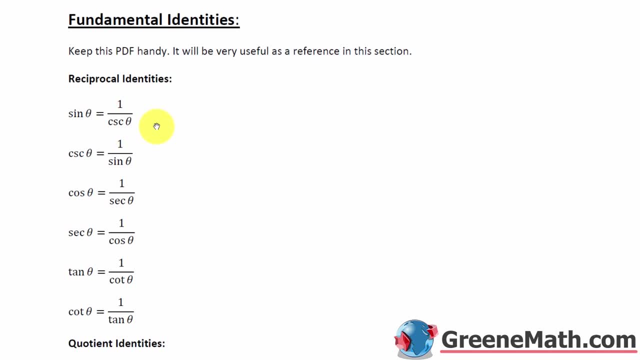 okay, as you get really good at working with these identities, you want to start by just going back and forth and reading things and writing it out. okay, as you get really good at working with these identities, you're going to commit these to memory. okay, You're really going to need to do this before. 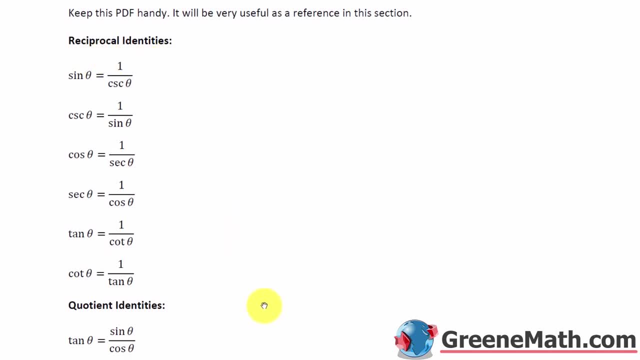 you get to calculus. So you have here the reciprocal identities. okay, We have here the quotient identities, We have here the Pythagorean identities and then the negative angle identities, which we just talked about. So we're going to use this in this section. 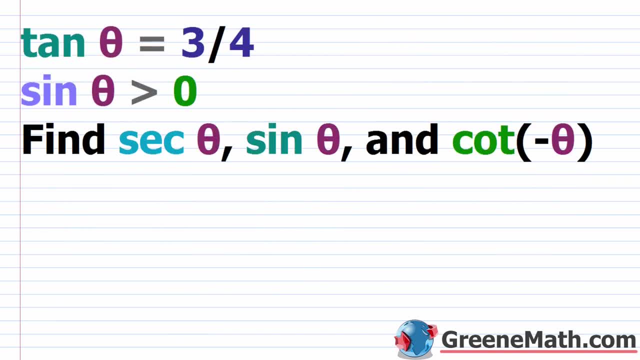 Together. these are all called the fundamental identities, And we're going to start by just solving a problem that we've already seen how to solve before. okay, We're just going to do it in a different way. So we have the tangent of: theta equals three-fourths and sine of theta is positive. 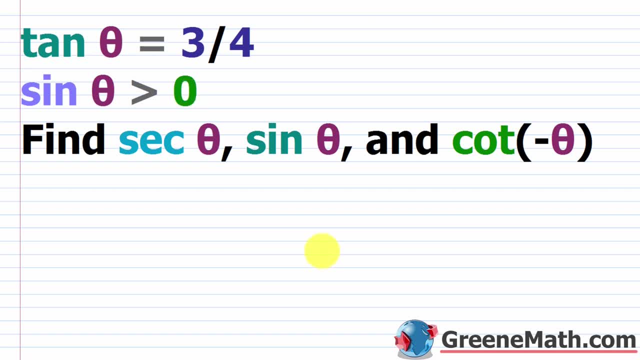 okay. So let's stop for a minute. This tells us we're where. Remember, the all students take calculus. So if I draw a little coordinate plane here, the all students take calculus. okay, Everything is positive in the first quadrant. In the second quadrant it's sine and cosecant. 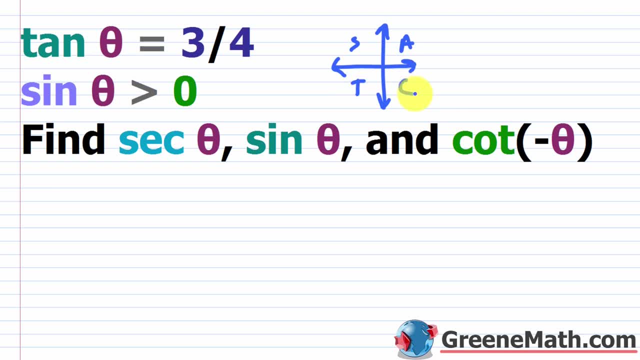 In the third quadrant it's tangent and cotangent, And in the fourth quadrant it's cosine and secant. okay, In terms of what's positive. So here we have that tangent is positive and so is sine. So that means I have to be in quadrant one, okay? So before you do anything, let's just figure. 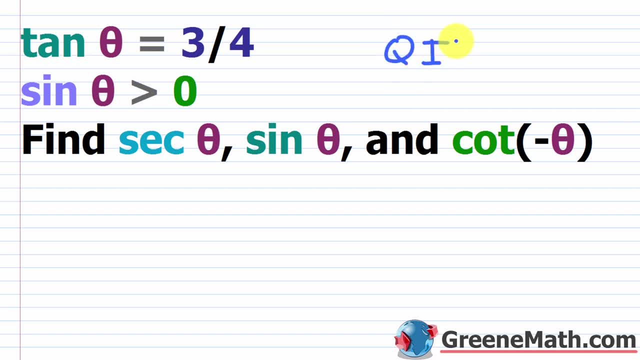 that out And we're just going to put here that we're in quadrant one. okay, So I want to find the secant of theta, the sine of theta and the cotangent of negative theta. So let's start out with the secant of theta. How can we figure this out using identities? Well, let me pop this back. 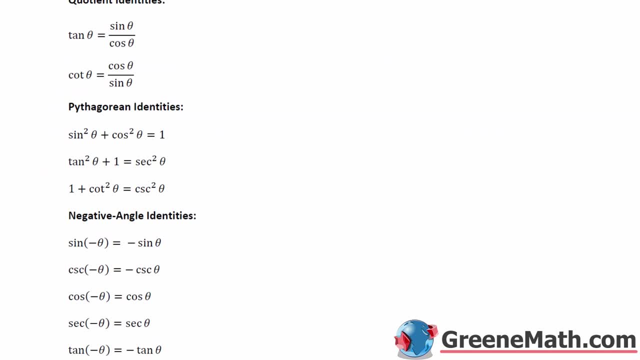 open and I want to look for a relationship between tangent and secant. okay, And I see that I have one here: tangent squared theta plus one equals secant squared theta, So let's go ahead and write this out. So we have that, the tangent. 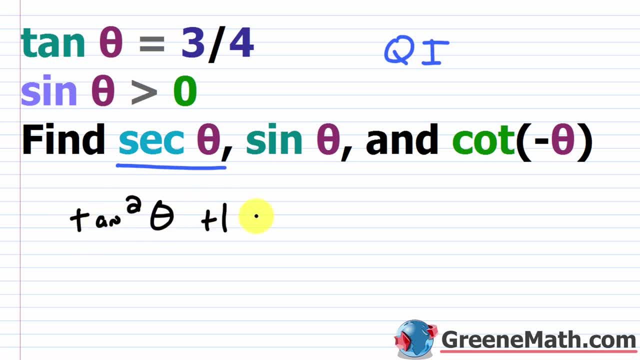 squared theta, Then we have plus one is going to be equal to the secant squared theta. okay, So remember- and this is going to come up later on, when we're simplifying trigonometric expressions- this is the same as if I had tangent theta squared. okay, This is just a different way. 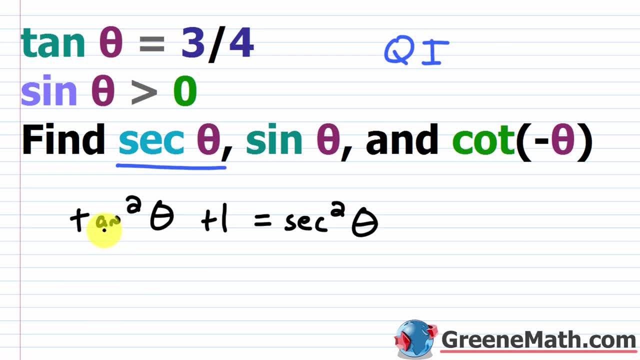 to write this. So what I'm going to do is I'm going to plug in, for what I'm going to do I'm going to. I have, So I'm going to plug in the three fourths there. This is three fourths and it's being. 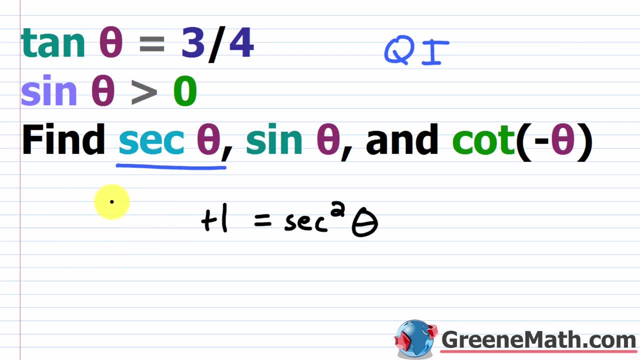 squared, Okay, That's why I just showed you that. So let's erase this and put three fourths here And I'm going to square this guy, Okay. And so if I square three fourths, I get nine sixteenths. 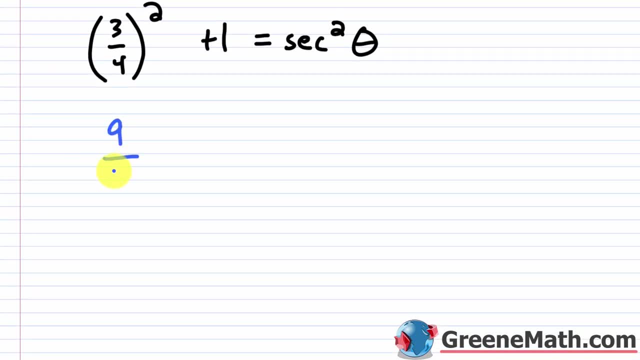 Let me scroll down and get some room going. We'll come back up and answer this. So this will be nine sixteenths plus one. Now, to do anything here, I know I need to get a common denominator, So I might as well just write this as 16 over 16 and just go ahead and add: nine plus 16 is 25.. 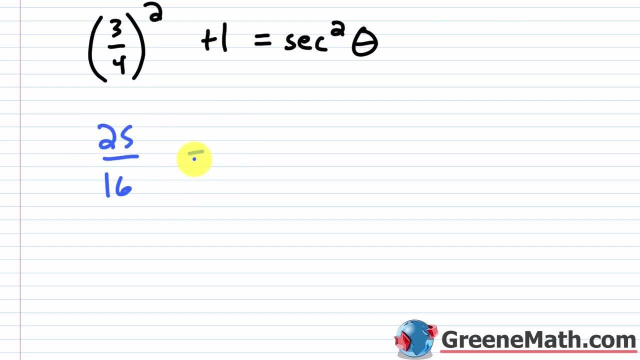 So this would be 25 over 16.. Okay, So this equals secant squared theta. Now I want to get this guy this secant of theta by itself, because that's what I'm told to find, right, I want to find: 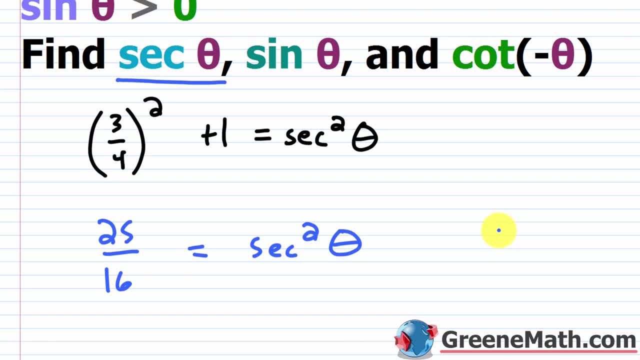 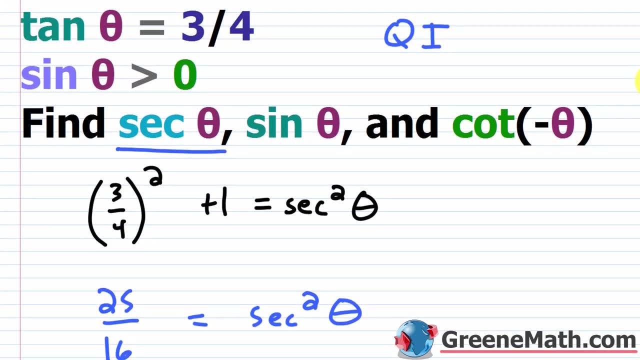 secant of theta, not secant squared of theta. So to do this, I want to take the square root, Okay, But I need to know which one to take And I need to think about: okay, well, if I'm in quadrant one. 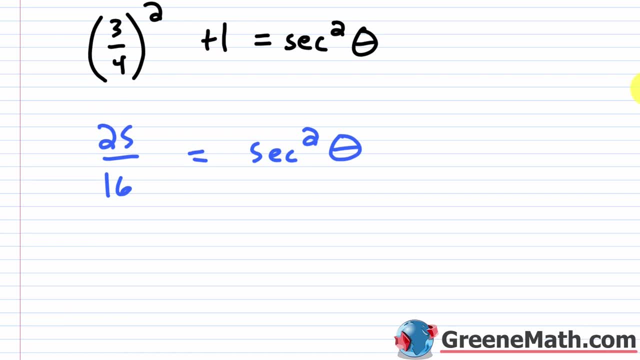 everything's going to be positive. Okay, So I just want the principal square root, So I'm going to take the principal square root. So I'm going to take the principal square root, So I'm going to square root over here, And this guy over here will now be just secant of theta. Okay, So here I. 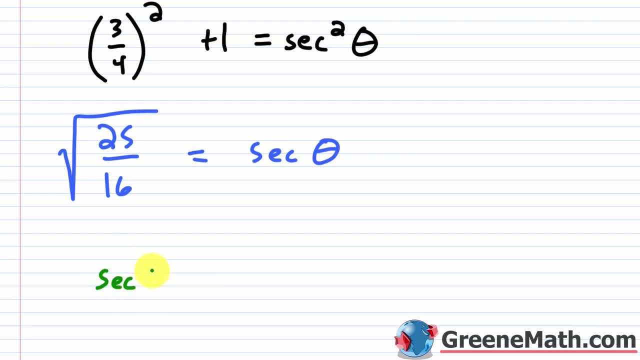 can simplify and say: and I'm just going to flip this around and say: the secant of theta is equal to the square root of 25 is five and the square root of 16 is four. So this guy is going to be five fourths. Okay. So that's one way we can do it. Obviously, we saw earlier in the course that 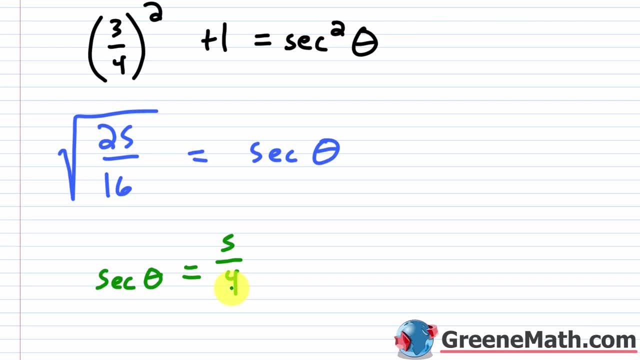 we could have done this a different way. whichever way you want to do it, I'm just showing you different ways you can attack the same problem. So let's put this up here, Let's erase all this and let's just drag this up here. 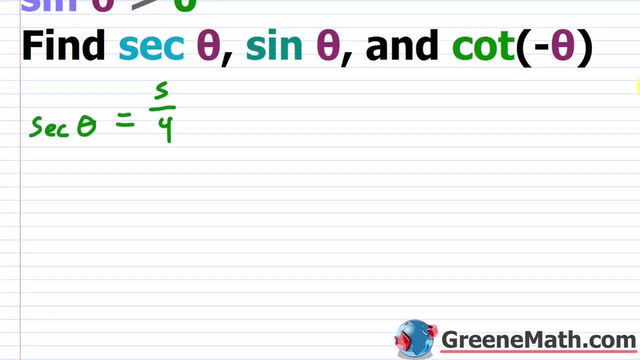 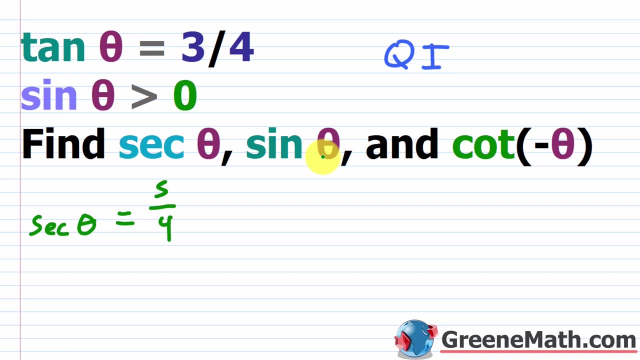 And we'll attack the next part of that problem. So we have here, we go on. come up here. We want to find the sine of theta, Okay. So let's think about this, And there's a lot of different ways to do this. But again, if I go back to my little cheat sheet, I want you to see this quotient: 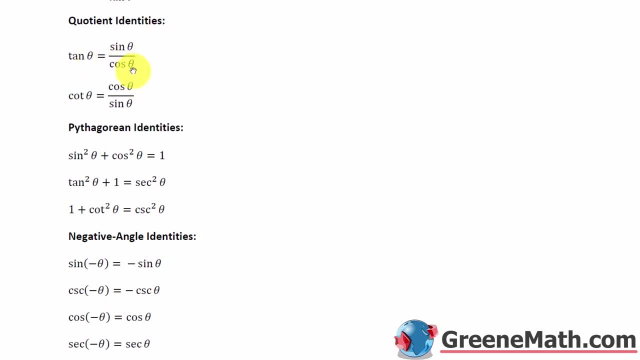 identity here, where the tangent of theta again is the sine of theta over the cosine of theta. Now you might think: well, we don't have cosine of theta, but we do because of the reciprocal identities. We just found the secant of theta, which is one over the cosine of theta. Okay, 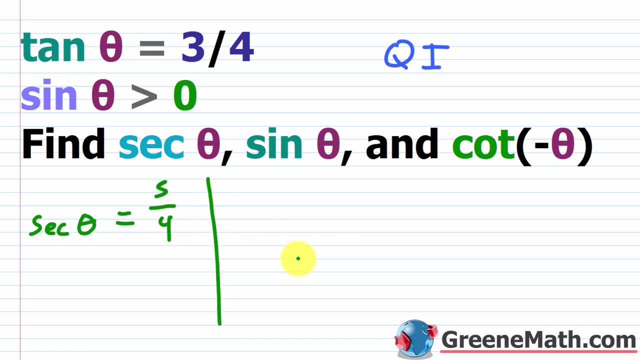 So let's go ahead and put this down here. I'm going to first just write the relationship: that the tangent of theta is equal to the sine of theta over the cosine of theta. Okay, And the cosine of theta is one over, So it's one over the secant of theta. Okay, So you know, you can flip. 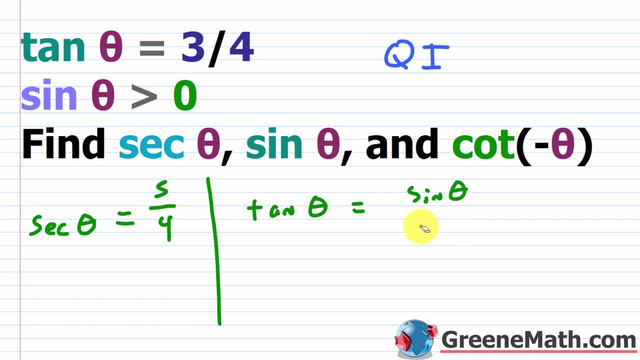 this and you would basically have the secant of theta. Okay Times, the sine of theta. but I want to solve for this guy, So I'm going to divide both sides by the secant of theta And that's going to give me the sine of theta by itself. Now all I have to do is plug in the. 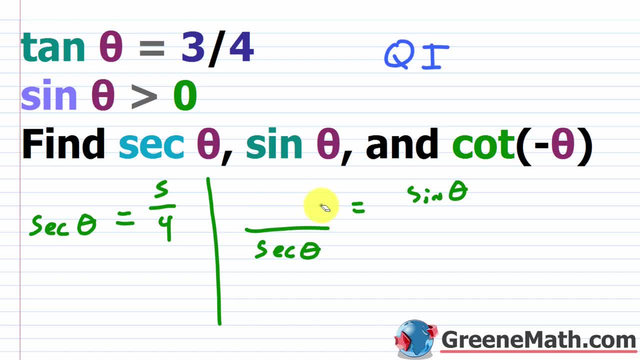 information I'm given. So I have for the tangent of theta three fourths. So I have three fourths for the secant of theta. I just found that was five fourths, Okay. So basically what I'm going to do here is say, let me scroll down and get some room going. I'll come back up. I have three. 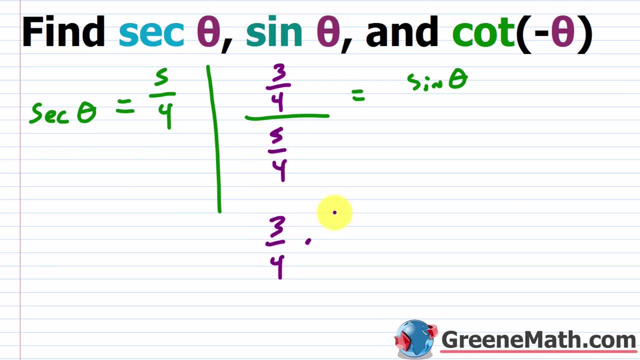 fourths times. I'm going to flip this because I'm dividing fractions. So four fifths, we can see this. So that's going to be my sine of theta. So let's go ahead and put this over here and say that my sine of theta is equal to three fifths. Okay, For the last part of this problem, we're. 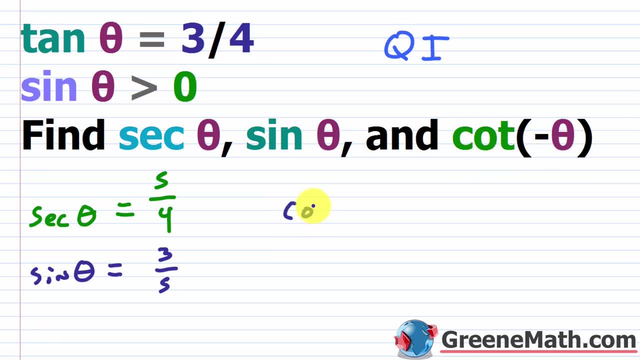 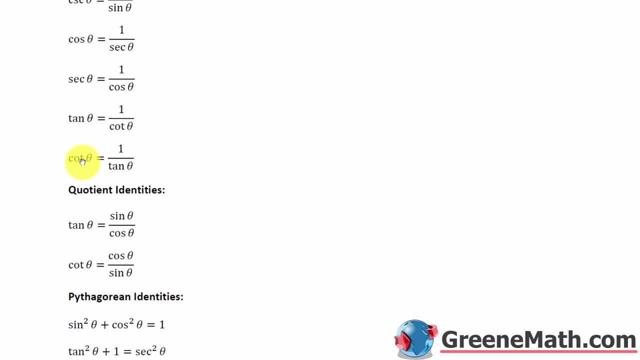 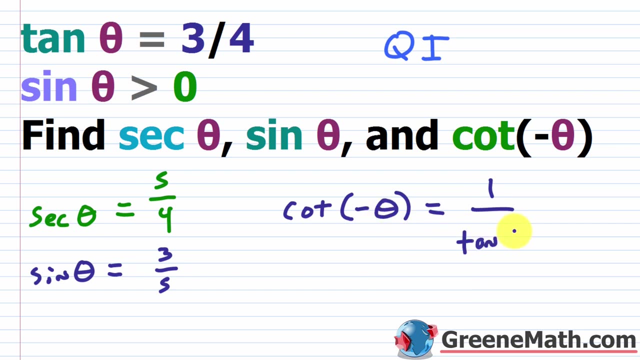 asked to find the cotangent of negative theta. So the cotangent of negative theta. Okay, Let's just pop open this guy again. We can see the cotangent of theta is one over the tangent of theta. Okay, So I could say this is one over the tangent. In this case I have a negative theta, So 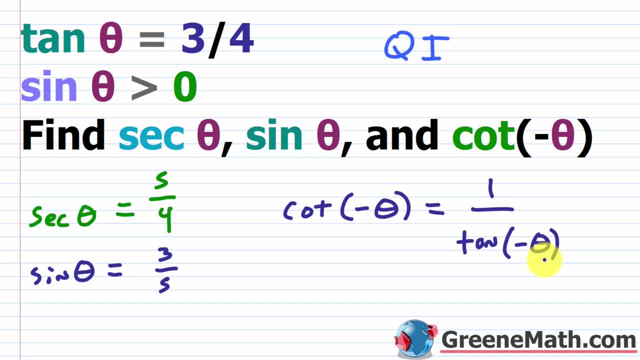 negative theta. Okay, And then from here I'm given that the tangent of theta is three fourths, but I want the negative of that, Remember you can pull this out. We saw that earlier. So you might as well say that this guy is going to be equal to one over the negative of three fourths. 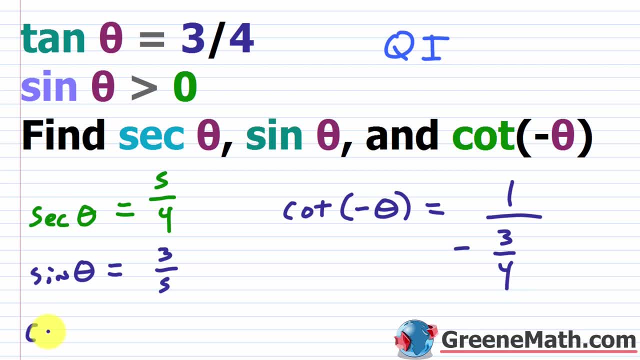 Okay. So to finish this up, I'm just going to flip this and say that the cotangent of negative theta is going to be equal to the negative of- again flip this guy. it would be four thirds. So those are going to be your answers here. Okay, You're going to have. the secant of theta is five fourths. 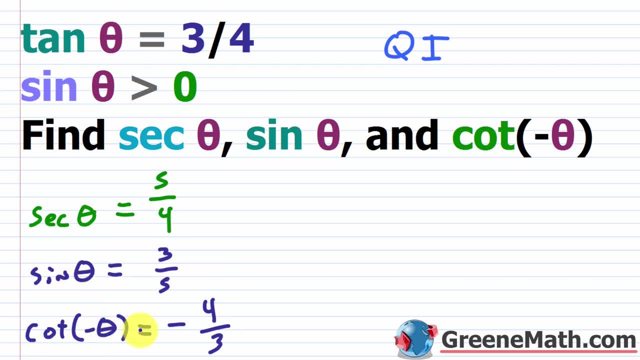 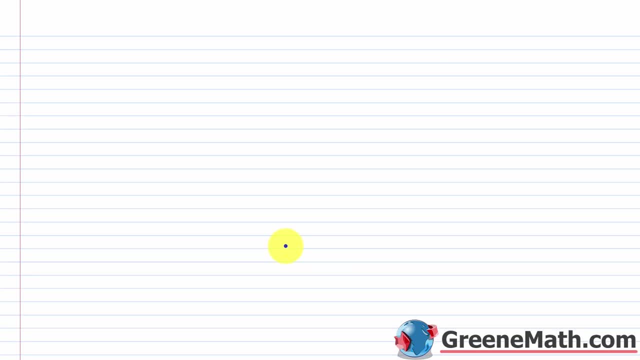 The sine of theta is three fifths and the cotangent of negative theta is negative four thirds. All right, So the next thing we want to do is we want to write one trigonometric function in terms of another. So you're going to see this in your book. Let's say you say something like: 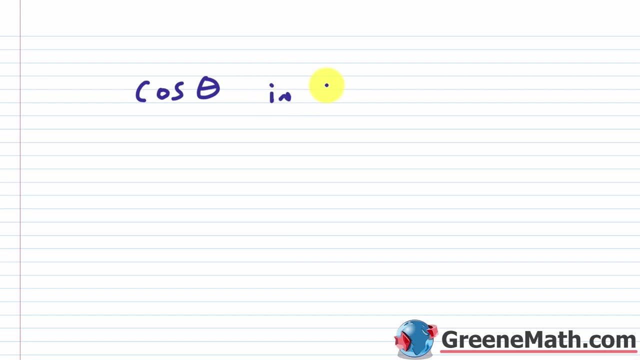 the cosine of theta, and you're asked to write this in terms of: okay, so in terms of the tangent of theta, Okay, So how can we do this? Well, what you want to do is you want to find an identity that's going to work where it's going. 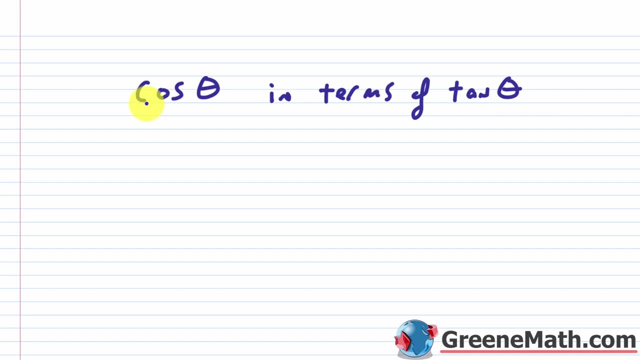 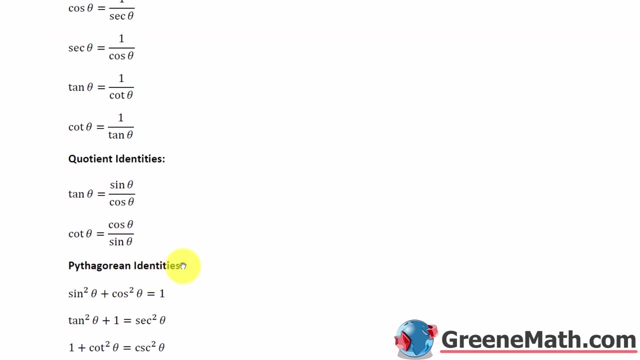 to relate your trigonometric function, which in this case is the cosine of theta, to the tangent of theta. So if we go back here, I'm going to pick this Pythagorean identity here, So I'm going to pick this guy which involves the tangent of theta, Okay, And the secant of theta. So what we're? 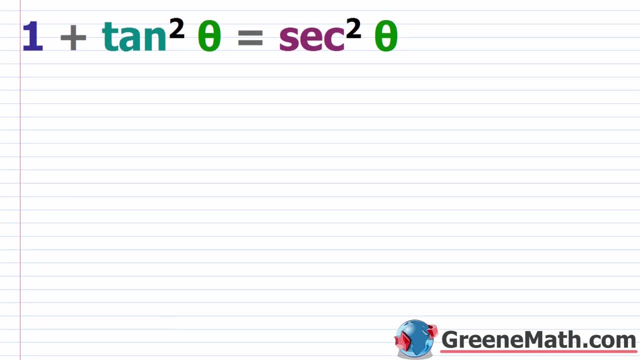 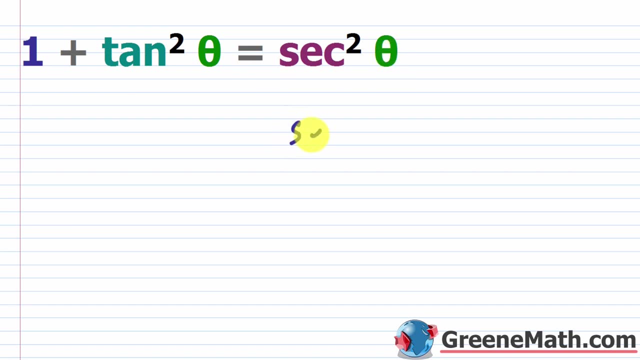 going to do? let's go ahead and minimize this. I'm going to go to the next page. I've already written it down. So we have one plus. the tangent squared of theta is equal to secant squared of theta. It's one over the cosine of theta, Okay, So what I'm going to do first is just take the. 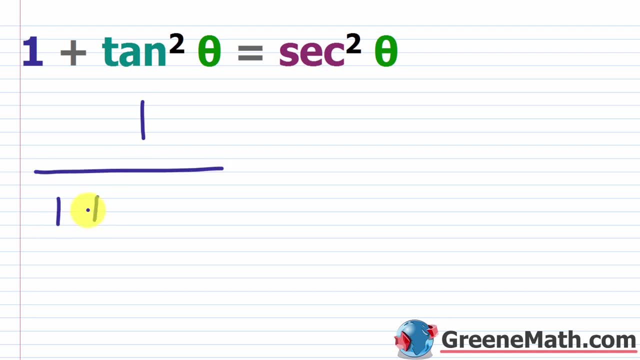 reciprocal of each side. So I'm going to say this is one over one plus tangent squared theta is equal to one over secant squared theta. Okay, So now I'm going to replace- I know that this guy right here again, because of the reciprocal identities, is going to be cosine squared theta- 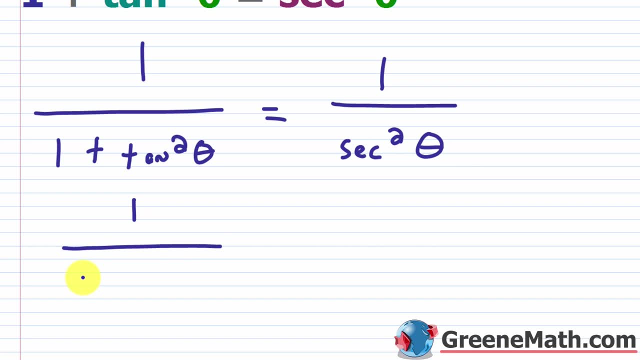 Okay, So I'm going to replace this. on the left, I'm going to say: one over one plus tangent squared theta is equal to. on the right, I'm just going to put cosine squared theta. Now, I want this in terms of cosine of theta. Okay, So I'm going to take the square. 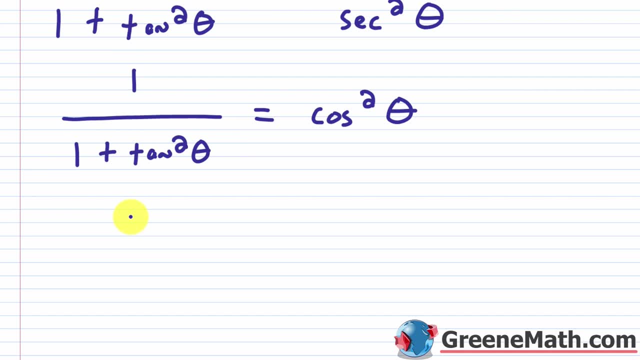 root of these sides here. on this side, I want plus or minus, because I'm not given a quadrant. Okay, So I don't know any information about what quadrant I'm in, So I'm going to write this. Let me change the color here I'm going to put. cosine of theta is equal to plus or minus. the square root of this. 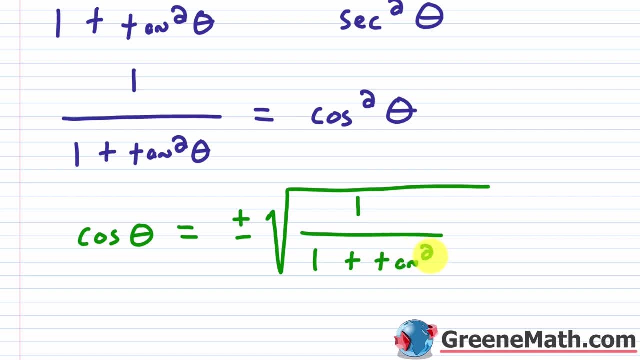 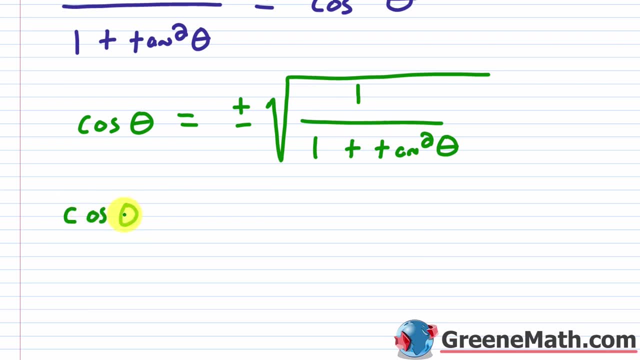 over. You've got one plus your tangent squared theta. Okay, So from here we know that we can take this and make it a one. So let's go ahead and say cosine of theta is equal to. I'm going to go plus or minus this one up here. over. down here I'll have the square root of one plus the tangent. 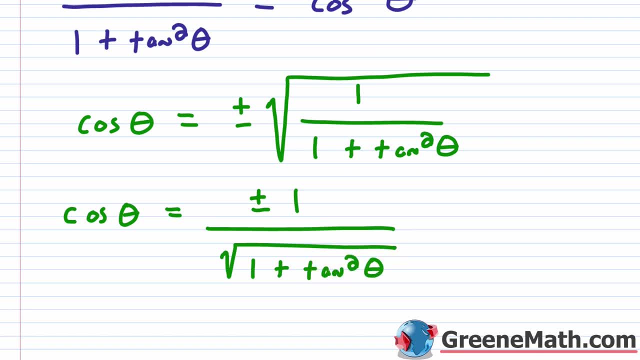 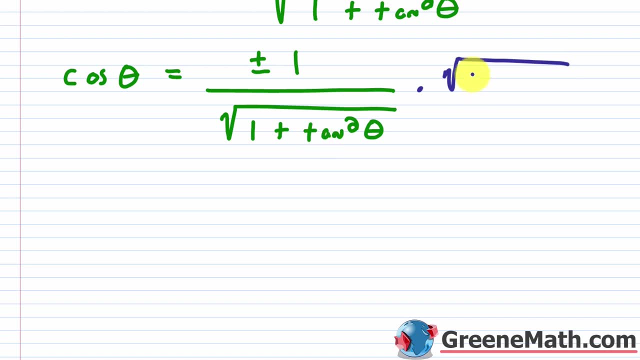 squared theta. Okay. So we want to always rationalize our denominator. So to do that, let me scroll down and get some more room going. I'm going to multiply this by the square root of one plus your tangent squared theta over square root of one plus your tangent squared theta- Okay. 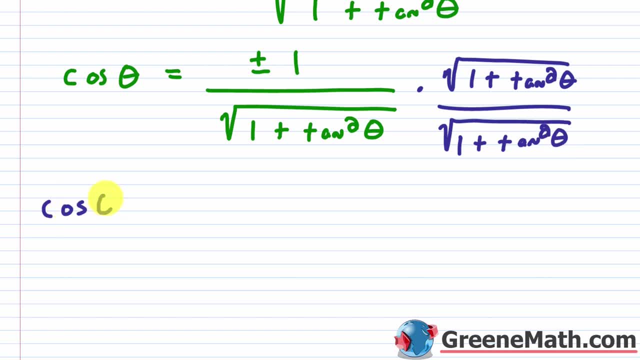 So that's just going to rationalize the denominator. So I'm going to have cosine of theta is equal to. So this guy right here. I'm just going to have plus or minus. Remember one times anything is just itself. So I'll have the square root of one plus tangent squared theta over this. 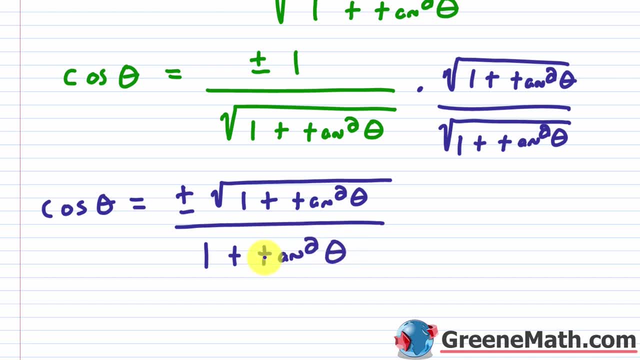 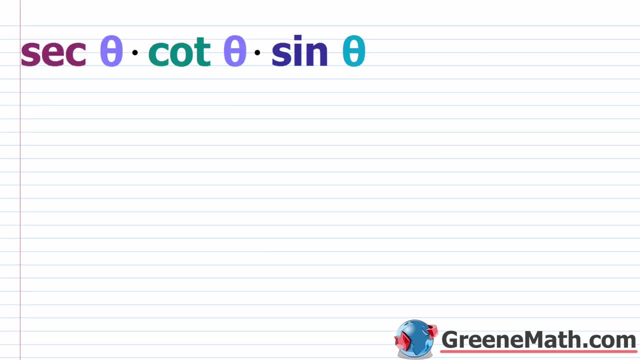 tangent squared theta. Okay, And we're done. So that's the exercise here. It's just meant to give you some practice writing one trigonometric function in terms of another. Okay, So now let's move into actually simplifying. Okay, And I think you'll find that once you get started on simplifying, 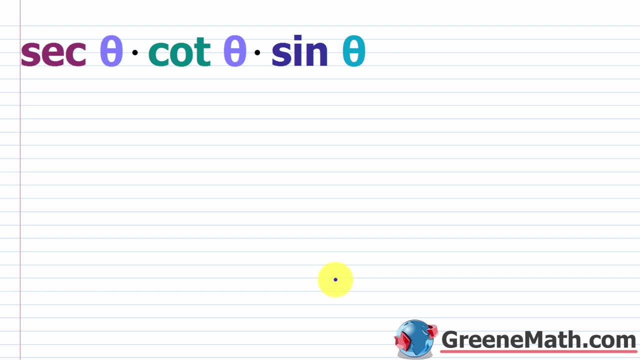 and writing things in terms of other things. at first it's a bit challenging, but really, once you practice enough, this becomes really really easy. So we have the secant of theta times the cotangent of theta times the sine of theta. So when you get a problem like this, you're going to 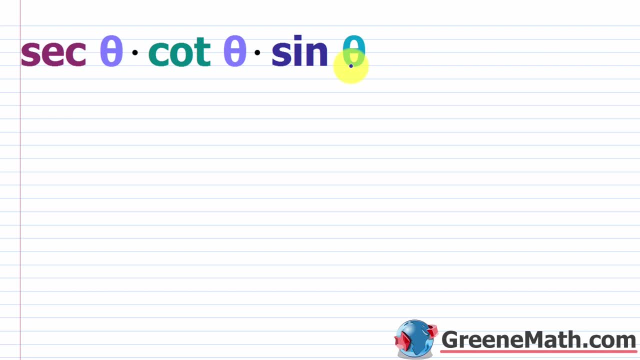 think about putting your expression in terms of sine and cosine. Okay, And if you have sine or cosine in your expression that you're trying to simplify, leave it alone, Don't try to mess with that. Okay, You want to mess with everything else, So I'm going to leave this as it is. 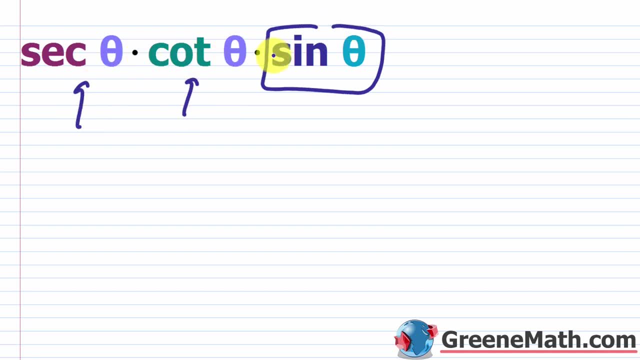 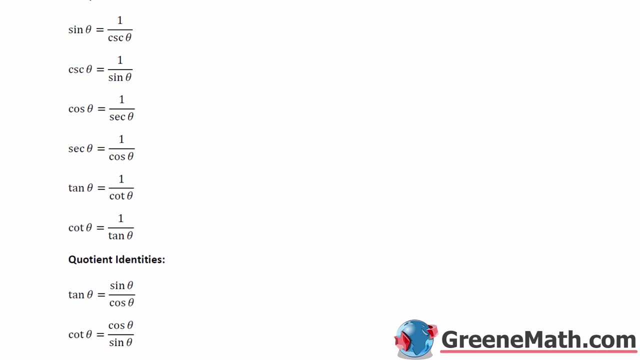 and I'm going to change this one in this one. So, because there's multiplication here, when I go back I'm going to be thinking about my reciprocal identities, Okay, So I'm going to be using these guys here to simplify. So, basically, the secant of theta is one over the cosine of theta, Okay, 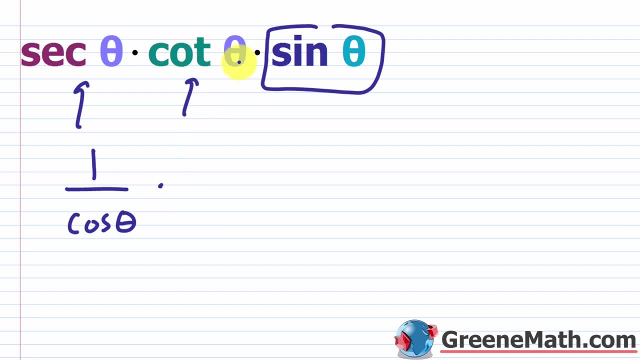 The cotangent of theta, I know is found by flipping the tangent of theta. So it's going to be the cosine of theta over the sine of theta, Okay, Over the sine of theta. And then this is times this sine of theta. So you see that when you plug these things in, a lot of stuff's going to. 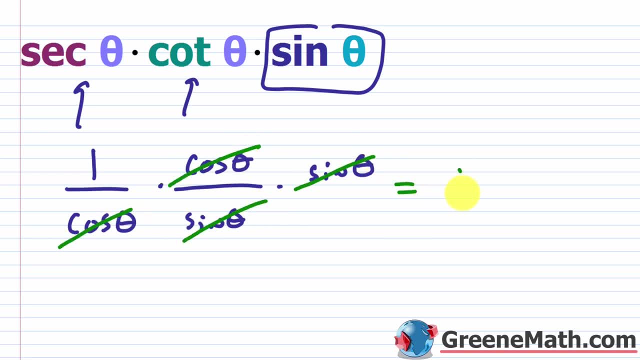 cancel. So this cancels with this, this cancels with this, and I'm basically just left with one, Okay. So this is pretty common When you just see multiplication like this: if you have sine or cosine, leave it alone. Okay, The other stuff is what you want to do, So you're going to leave it. 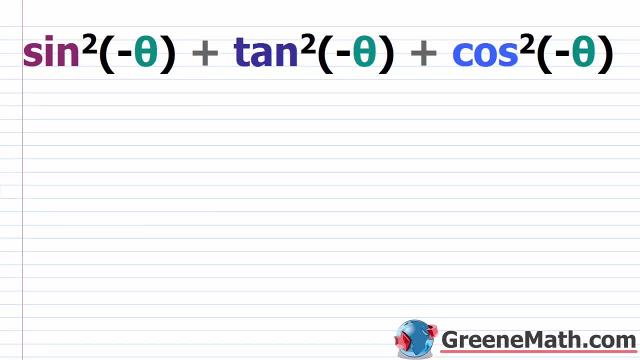 alone You're going to plug in for and try to see what you can get to cancel. Let's take a look at another example where we're simplifying a trigonometric expression. This one is going to be problematic for a lot of beginners because of the notation here, So I want to make sure you 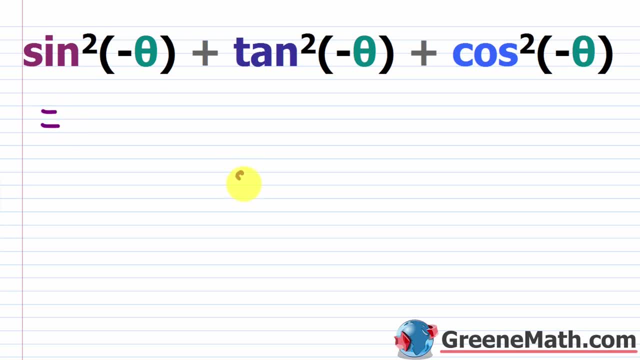 understand the notation. So when we work with again something like sine squared theta- remember this is the same thing as if I said sine of theta being squared like this. It's very important you understand that When you look at this guy right here, the temptation because of 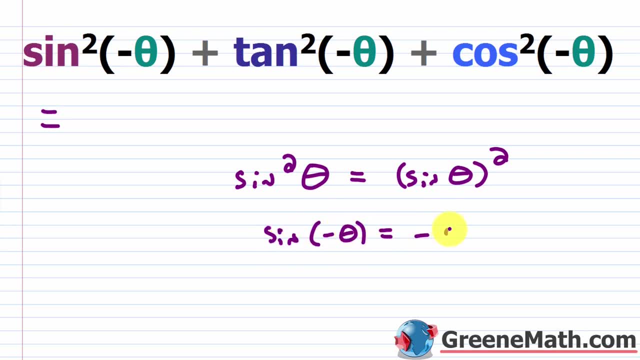 sine of negative theta- okay, is equal to the negative of the sine of theta. The temptation here is to do what It's to go: the negative sine squared theta- Okay. That's not actually accurate. Okay, You have to think about it like this, like this guy right here, Okay. So the way I want to. 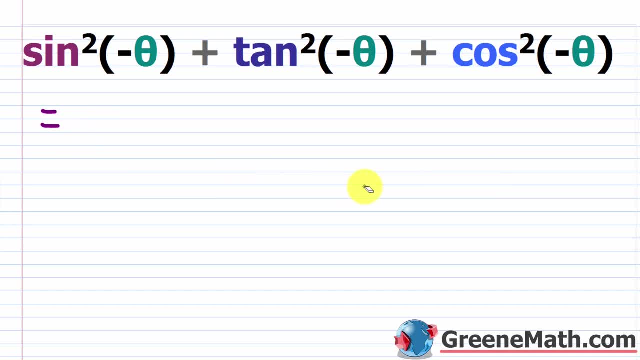 write this is. I want to make it crystal clear what's going on And I want to say that I have the sine of negative theta: Okay, This guy being squared, Okay, The whole thing being squared. Then, plus, I'm going to do the same thing here, So I'm going to have the tangent of this negative. 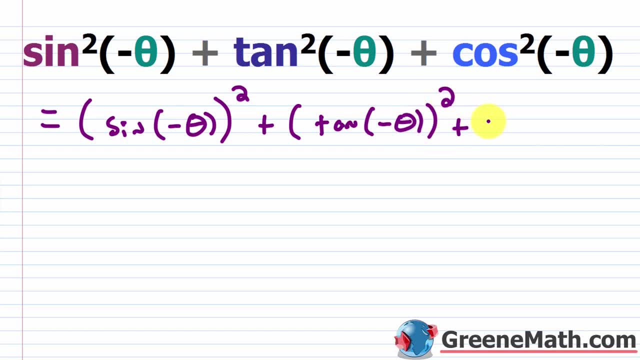 theta: Okay, This guy right here being squared. Then, plus, I'm going to have the cosine of this negative theta being squared, Okay, The whole thing being squared. So now it's crystal clear. Okay, When I pull this negative out, what's going to happen? We're going to have the negative. 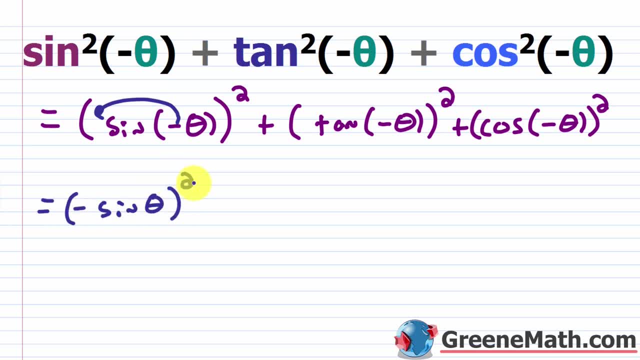 of sine of theta. but the thing is squared, Plus, pull this out. Okay, I'm going to have the negative of the tangent of theta and I don't need parentheses in that case. Okay, And then this guy's going to be squared, And then, plus, in this case, you don't need to pull. 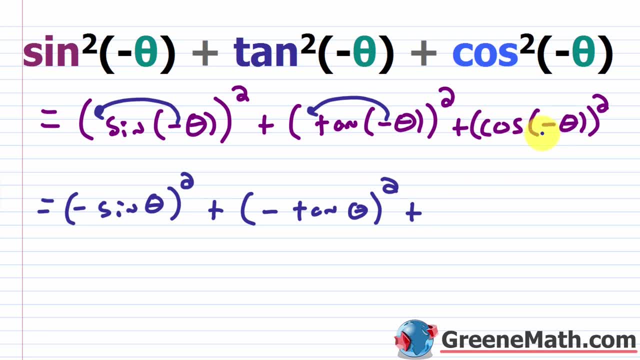 anything out, because the cosine of negative theta is equal to cosine of theta. Okay. So I can just say this is the cosine of theta being squared, Okay. So now I want you to see what I'm getting at here. Basically, if you had incorrectly pulled that out and said you had the negative, 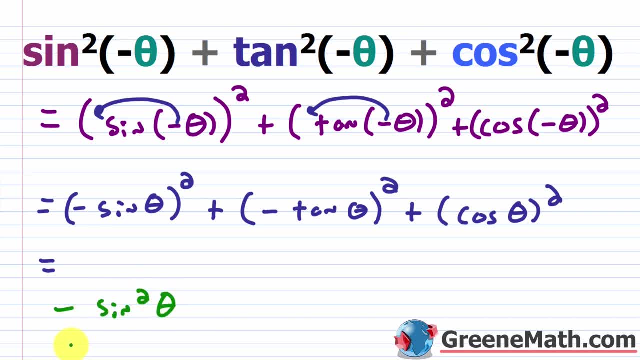 of sine squared theta, you would get the wrong answer. Okay, Because this guy right here: if you're squaring the negative, it becomes positive, right? So this is going to go away. So you get rid of that and you basically go back to having sine squared theta Not. 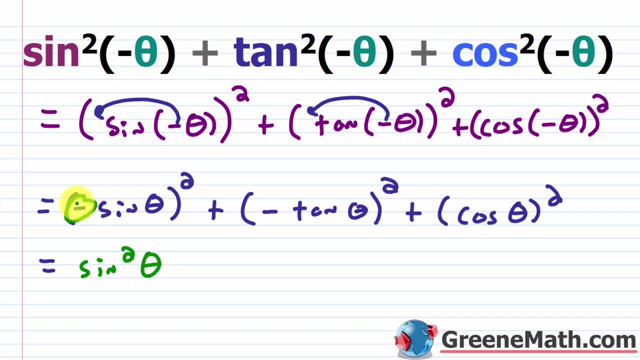 the negative of sine squared theta. sine squared theta. Okay, Because this negative got squared. Same thing here. This negative is going to get squared. So plus tangent squared theta, Then, plus you have your cosine squared theta, Okay. So from here, that's the first step. 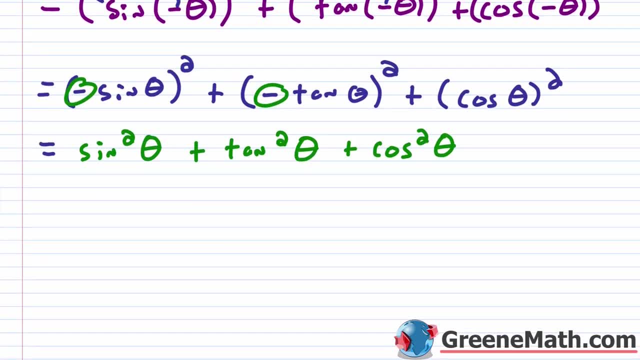 just to understand where you're going there. But from here you want to realize that if you're dealing with something that's squares here and you've got pluses and minuses involved, not in every case, but usually you want to look at the Pythagorean identities. So we 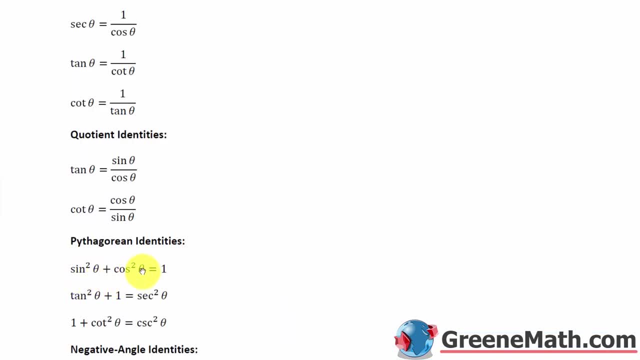 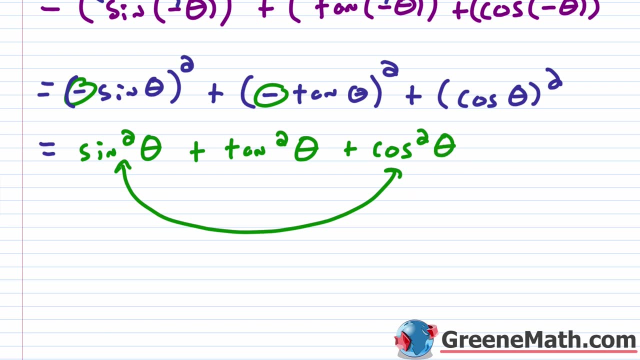 pop these open. You see that sine squared theta plus cosine squared theta is one. So that's the first thing I'm going to do. You can consider this plus this to be one. You can reorder this if you want to make it crystal clear. So we'll say sine squared theta plus. 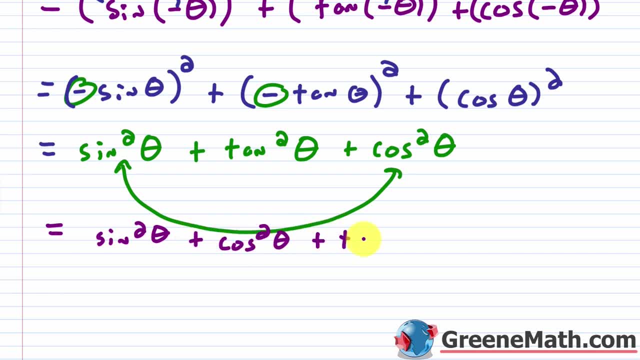 your cosine squared theta plus your tangent squared theta. Okay, This guy right here is equal to one. Okay, We just saw that, So I'm just going to substitute. So I'm going to put in here a one plus the tangent squared theta. Now can we make this? 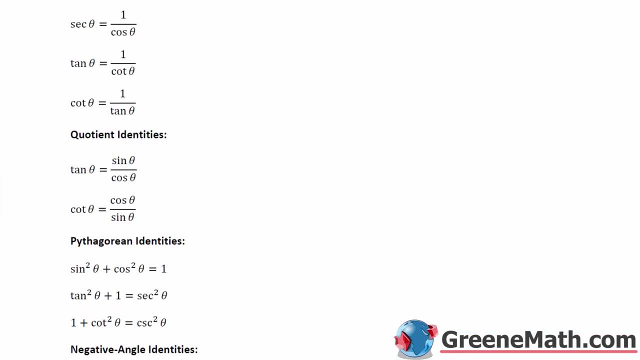 simpler. Let's go back and see if there's anything that involves tangent squared theta and one. Yes, right here. Tangent squared theta plus one is equal to secant squared theta, So I can replace this with just secant squared theta. Okay, And that's going to be. 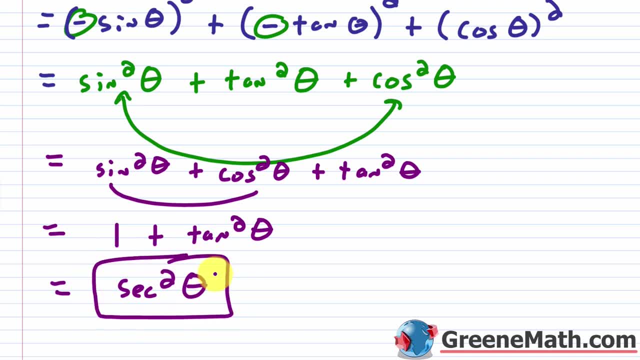 my answer And you can see how we really simplify this down to just one of these guys. So I'm going to put in here a one plus the tangent squared theta plus one. So that's what we're going to do. So what you might think is a good idea is you might want to go back and 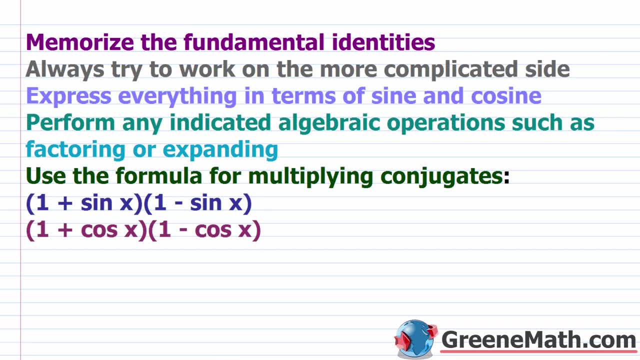 look at the table in the middle and look at the table that you're using to get the right answer. But in this lesson we want to talk about verifying trigonometric identities, All right, So in this particular section you might struggle a little bit when you first. 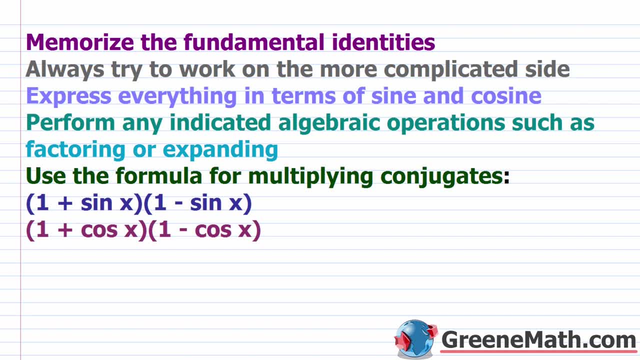 get to it. It's a topic that you really need a lot of practice with. It's not as straightforward as other topics, where you have a set list of things that you need to do. Okay, If you were solving basic equations, I could give you the steps and you could perform those. 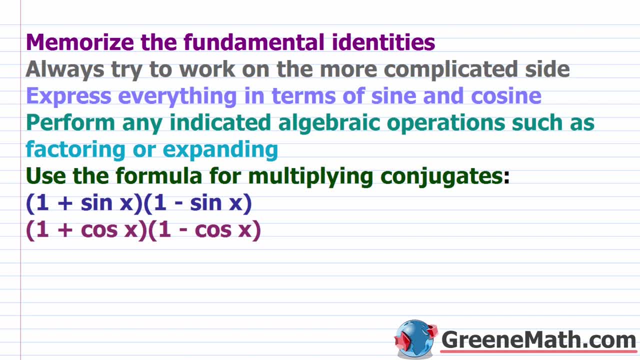 steps and basically you would get the right answer all the time. With this there are just hints or strategies you can use to get the right answer, And you can also come up strategies you can use to arrive at the correct answer, But it's not so clear in terms of what 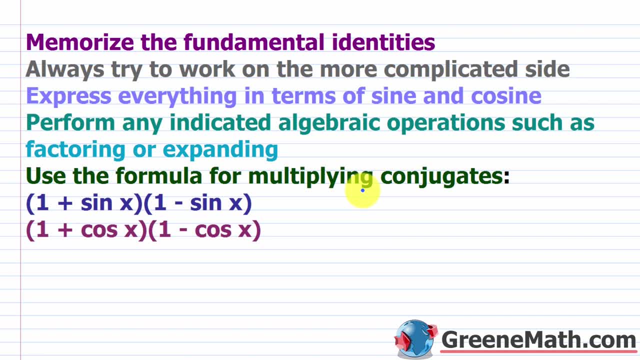 you need to do, And there's also multiple ways to do the same thing. Okay, so I have some little tips here for you, And they're standard from any textbook. Okay so you'll get this in any textbook. The first thing is to memorize the fundamental identities. So, again in the last lesson, 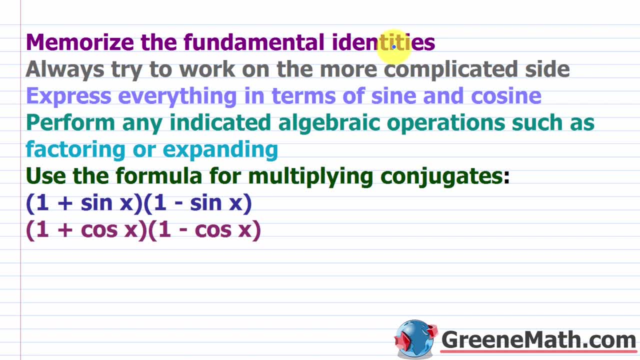 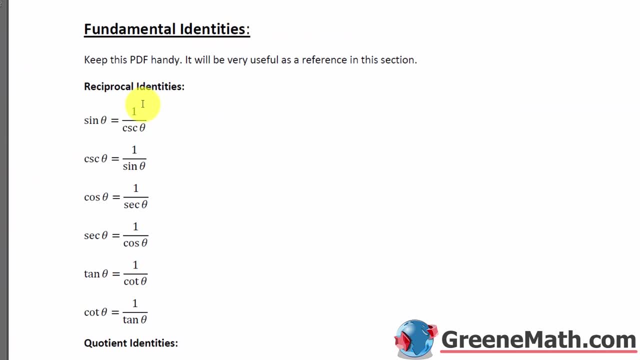 we talked about these fundamental identities. we talked about simplifying trigonometric expressions using the fundamental identities. Again, we looked at a little handout here, So hopefully you have that again And you want to memorize these. So you have the reciprocal identities. 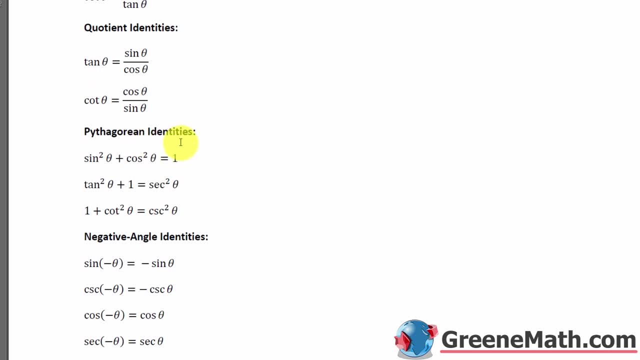 you have the quotient identities, the Pythagorean identities, and then you have your negative angle, or, again, some books call this even odd identities. So all of these are going to play a crucial role when you're verifying these trigonometric identities. Okay, so here are some other tips. 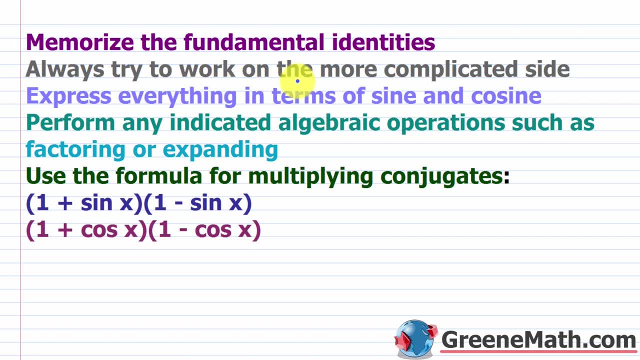 you always want to try to work on the more complicated side. Okay, so when you're verifying trigonometric identities, you're not going to be doing the same thing, So you want to work on the more complicated side and try to make it match the other side. 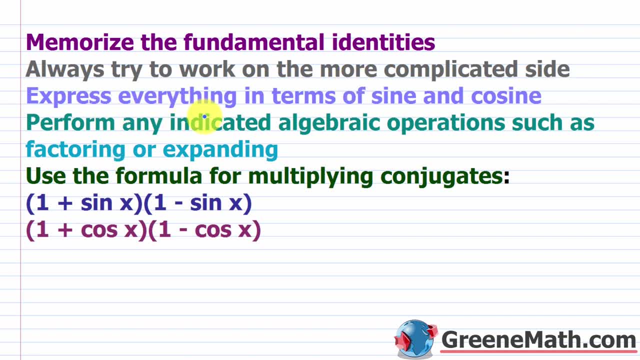 the simpler side, Okay. Another tip is: sometimes you'll want to express everything in terms of sine and cosine. That doesn't always work, but it's just a general tip. Okay, you want to perform any indicated algebraic operations, such as factoring or expanding. Here you want to think: 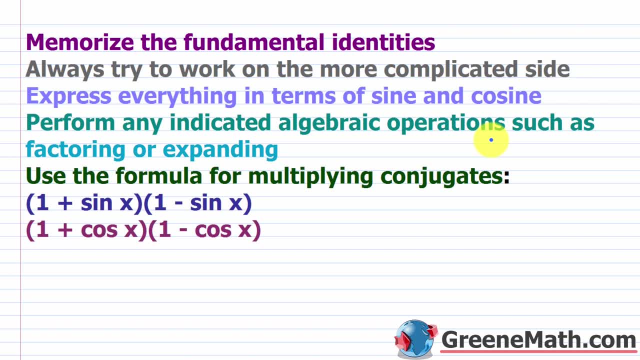 about all those special product formulas, okay, and all the special factoring formulas. those are going to come up a lot. And then we have use the formula for multiplying conjugates. So remember, if you have one plus sine of x times one minus sine of x, this is going to be one. 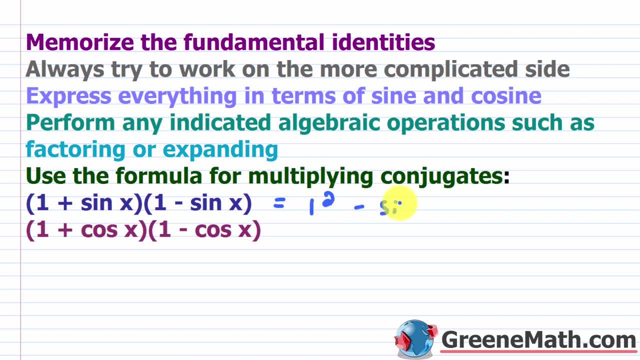 squared, which is one, and then minus sine squared x. So basically one minus sine squared x, And we know from our Pythagorean identities this is going to be exactly equal to cosine squared x. Similarly, here I could make this one minus cosine squared x. okay, and that's going to be. 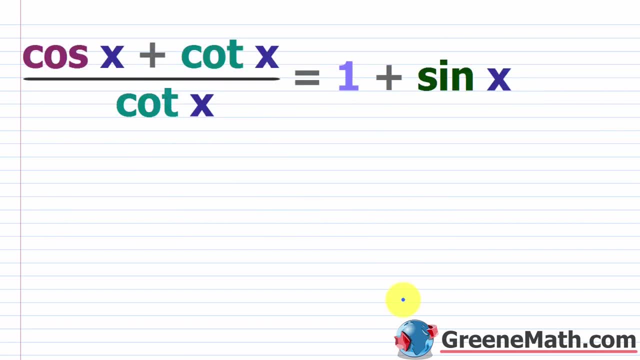 exactly equal to sine squared x. Okay, so let's take a look at the first example, And the first few of these are going to be really, really easy. So go ahead and pause the video and try them on your own Once I kind of get going here and then see the solution. So the first thing is I'm going 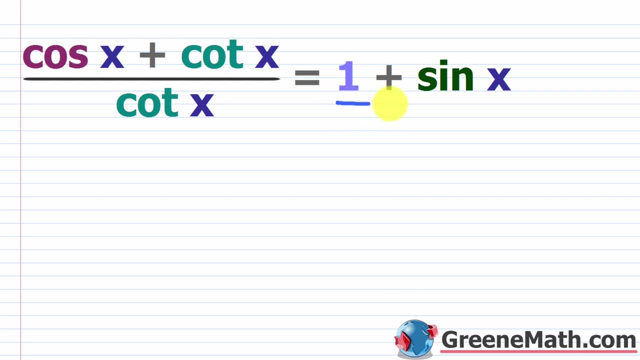 to think about which side is simpler. So to me this side is simpler, Okay, so I'm going to try. left Now, pretty much every book that you're going to see has different formatting. Generally speaking, they sometimes will take this guy right here and just work on the more complicated side. 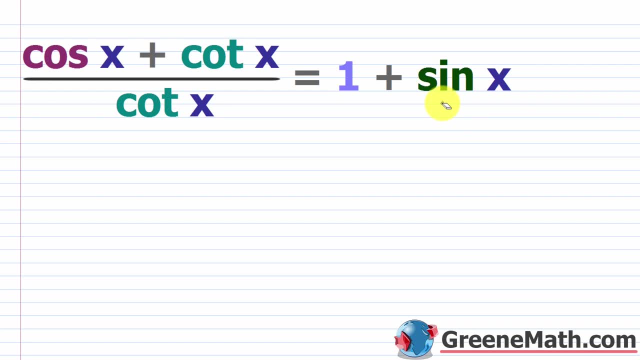 And the end. they'll show you that it matches. What I'm going to do here is I'm just going to take this guy and flip it. So I'm just going to say I have one plus sine of x is equal to. over here I'm going to have cosine of x plus cotangent of x. okay, over the cotangent of x I'm flipping. 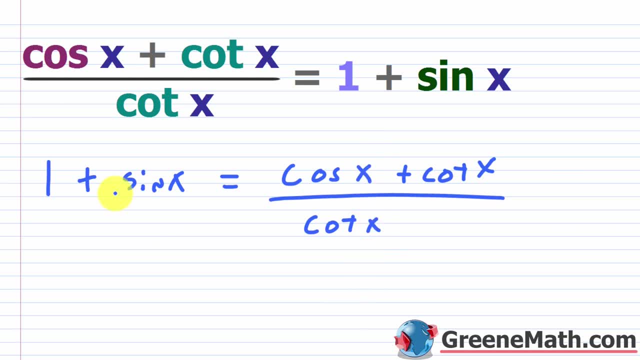 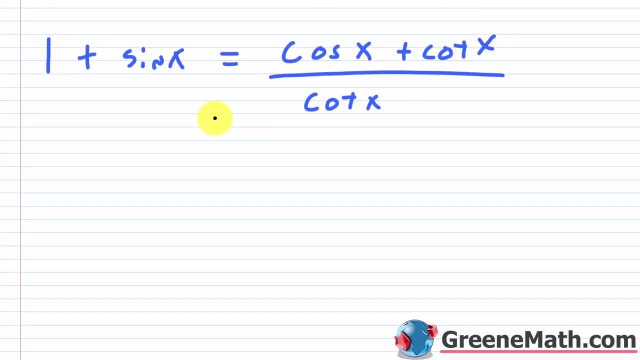 over here and I'm going to have cosine of x plus cosine of x plus cosine of x plus cosine of x. So that's generally the formatting you're going to see. if your teacher tells you to do something else, then follow that, Okay. so what I'm going to do is just put equals over here. I'm not going to mess. 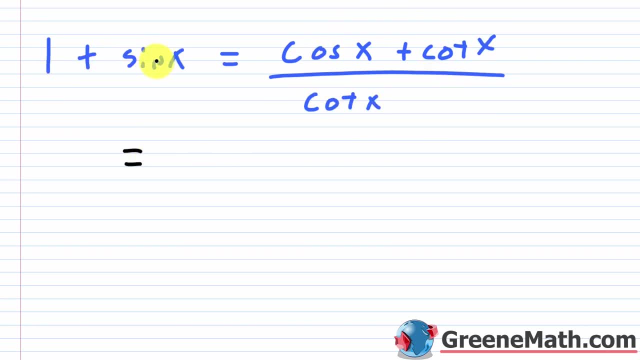 with this. my goal is to get this side right here to match this one plus sine of x. So the first thing I'm going to do is I'm going to write things in terms of sine and cosine. So I have cosine here, okay, so I'm not going to touch that- But cotangent of x again, if you think about the reciprocal. 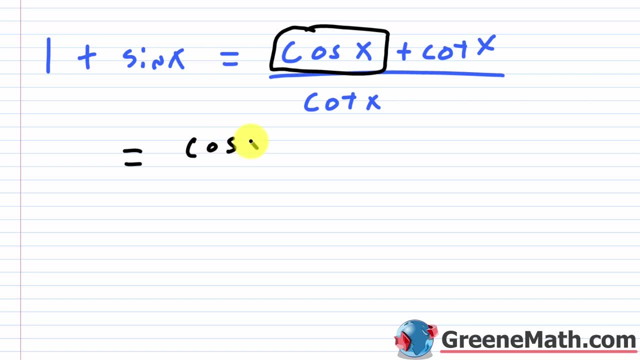 of x over sine of x. So I'm going to start by saying I have cosine of x plus cosine of x over sine of x, And this is over again. if I have cotangent of x, I'm going to write it as cosine. 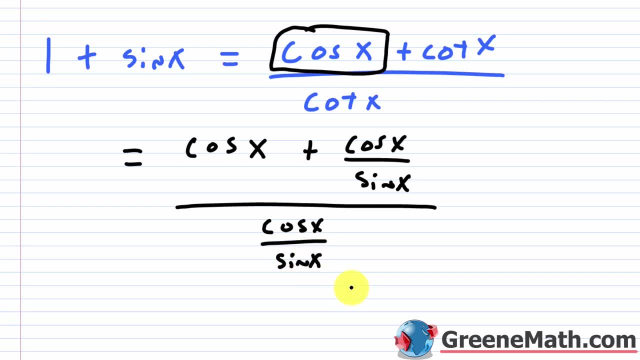 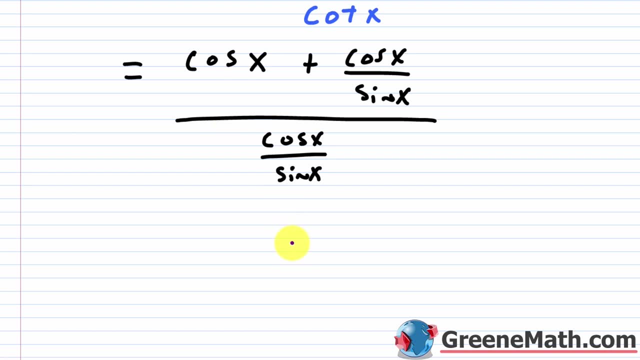 of x over sine of x. Okay, let's go down and get some room. we'll come back up when we get to a stopping point, Okay, So what I want to do here is think about the fact that I have basically a complex fraction, right? So how do you simplify that? You look at the denominator, so I have sine. 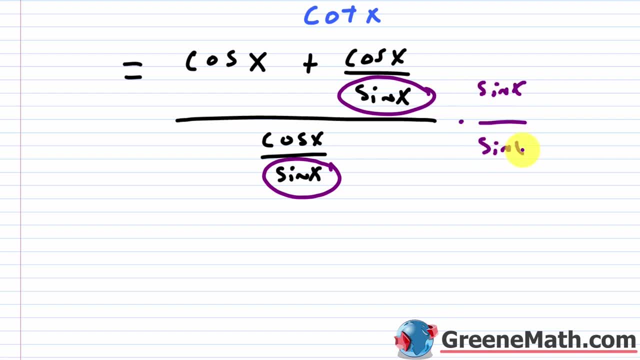 of x over cosine of x. So if I multiply this by sine of x over sine of x, basically I'm going to distribute this here and here. okay, and I'm going to distribute this here, So I'm just going to keep. 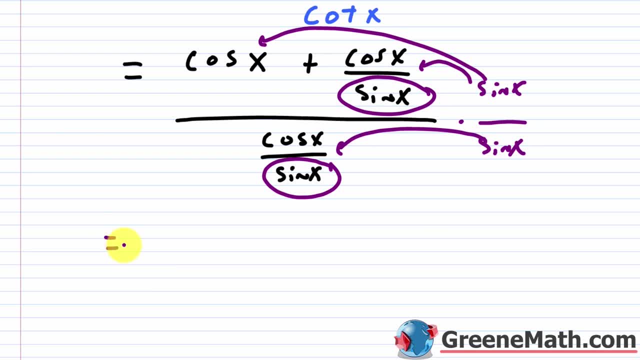 my equals over here. Okay, we might need more room, So let me just kind of slide this down a little bit. Sine of x times cosine of x is just sine of x times cosine of x, then plus sine of x. here we cancel with sine of x here, So I just have cosine of x here. Okay, then down here this: 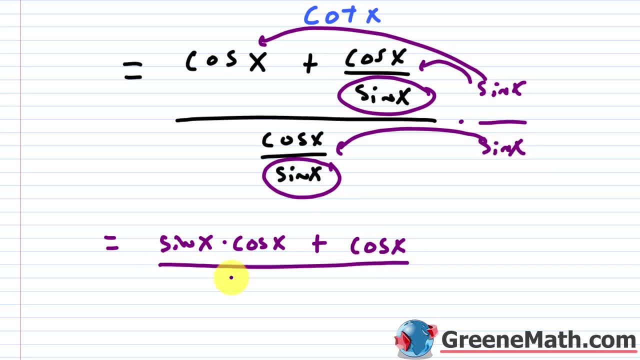 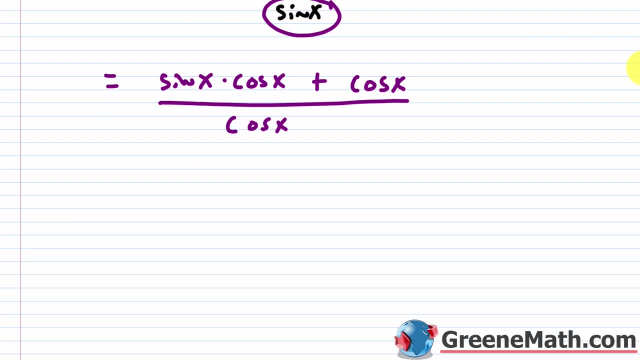 sine of x here. we cancel with this sine of x here. So I'm going to put this over Just the cosine of x. Okay, so let's go down a little bit more And let's think about something. here We have the cosine of x and the cosine of x. what operation could I do there? Well, 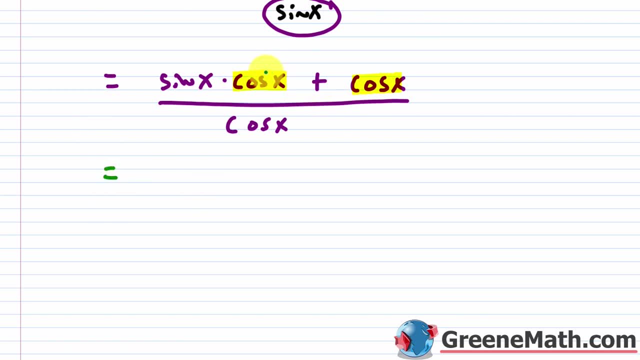 I could factor right. So I'm going to put equals here And I'm going to pull that guy out. Okay, so I'm going to say I have the cosine of x Inside the parentheses, I'll have the sine of x. 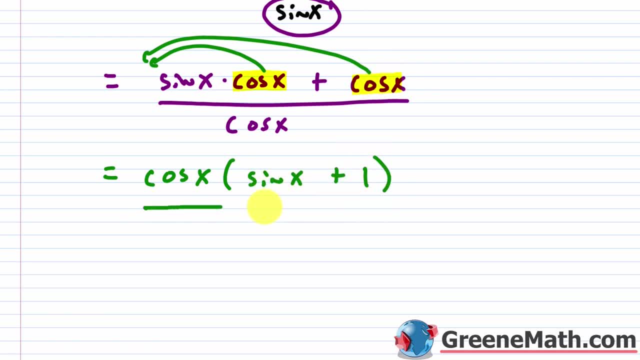 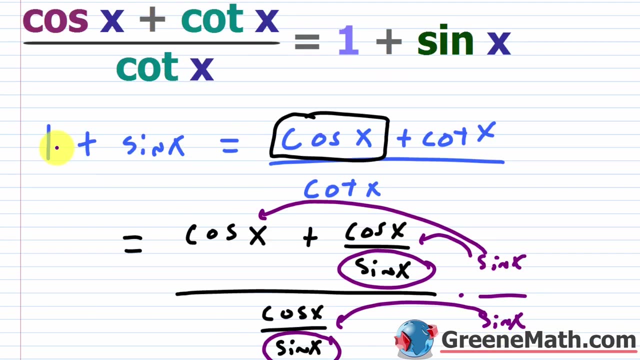 okay, plus, if I pull this out, I have a one. okay, then this is over the cosine of x. And now what I'm going to do is I'm going to cancel this with this And what I'm left with is going to be the sine of x plus one. Okay, if we go all the way back up, we see here that we have 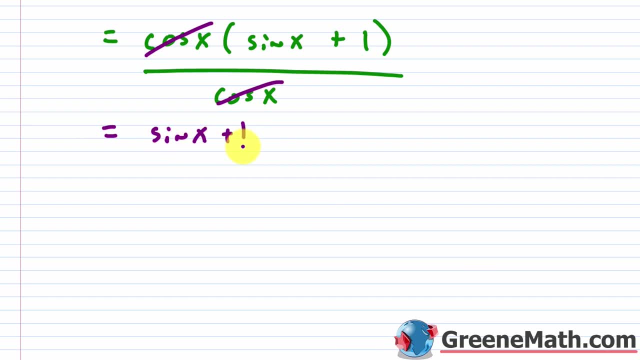 one plus sine of x. In here we have sine of x plus one right, So I could write this as one plus sine of x. Okay, And then I'm just going to put a big checkmark here to show that this right side. 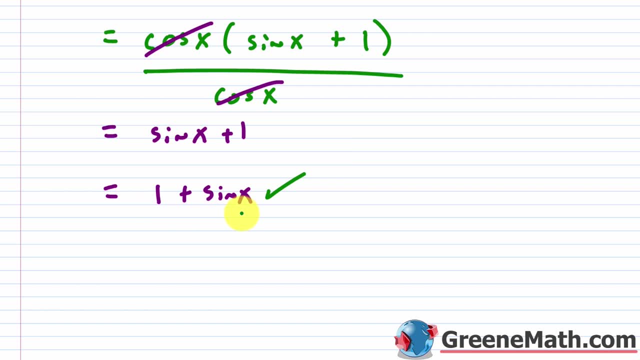 now, here matches the left side. Okay, So you could have gone about this a different way. There's multiple ways to do this, But I'm going to put a big checkmark here, And I'm going to put a big checkmark here. So if you want to verify a trigonometric identity, the main thing is: 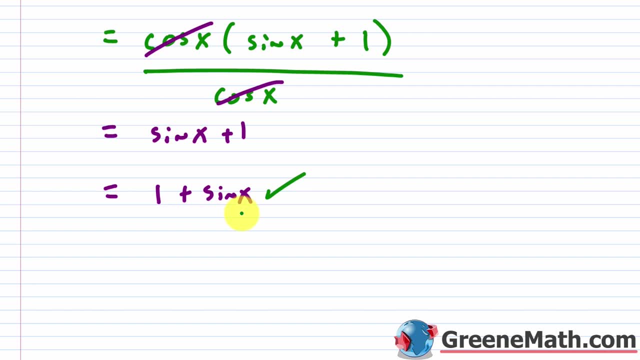 again. start with the more complicated side, work your way down- okay, and try to make it match the other side, Okay. so once you've found that it matches, you're done, put your checkmark and move on. Try to make your steps as clear as possible so that whoever is grading it can give. 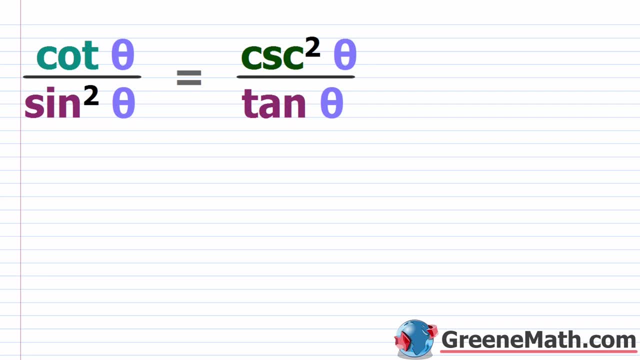 you full credit. Okay, let's take a look at another example. This is another kind of easy one. So we have the cotangent of theta over sine. squared theta equals cosecant squared theta over tangent of theta. Now, in this particular case, both sides are equally complex, So I'm just 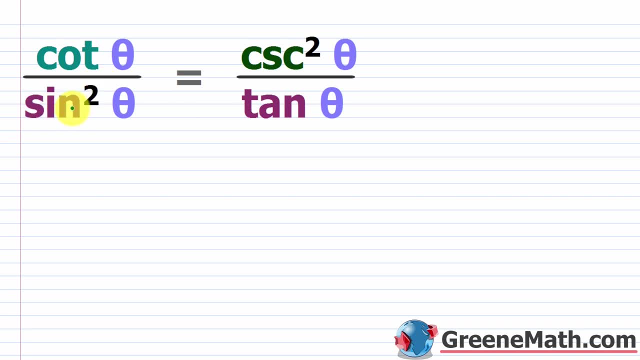 going to leave the left one alone because it already contains sine. okay, If you wanted to do it a different way again, that's fine. So I'm just going to basically put equals here And I'm going to manipulate this in terms of sine and cosine, So cosecant. okay, if I think about the 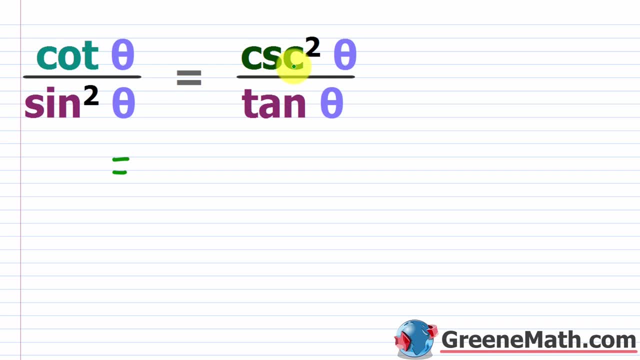 reciprocal identities is one over sine, okay. So basically I can say: cosecant squared of theta is one over sine squared of theta, okay. And then over tangent of theta is going to be my sine of theta over my cosine of theta, okay. So what I want to do here, think about the fact that you 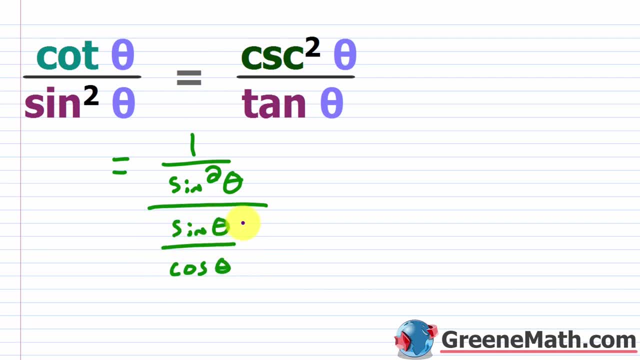 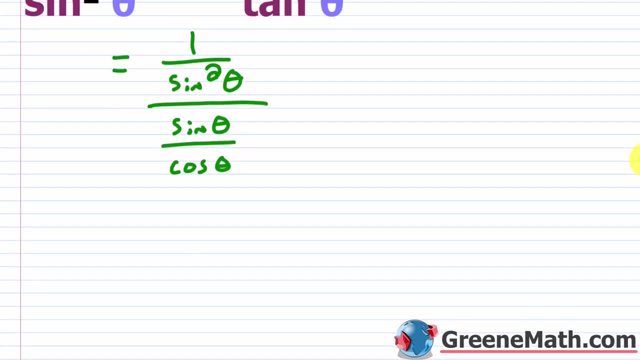 are basically going to flip this guy. okay, Basically, if you're going to divide fractions, you multiply the first fraction by the reciprocal of the second guy. okay. So let's scroll down a little bit And I'm going to go one over sine. 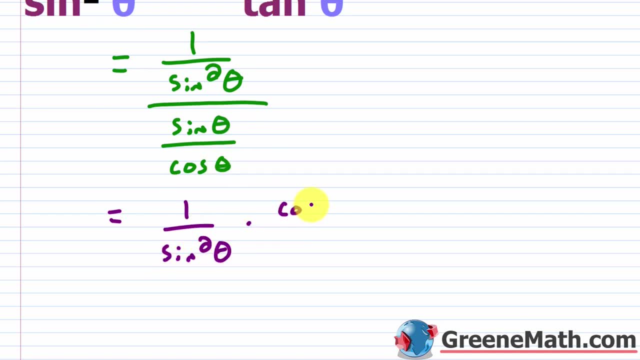 squared theta times. this is going to flip, so it's going to be cosine of theta over sine of theta. okay, And can anything cancel here? Well, no, you might be expecting to cancel sine of theta. So at this point you might stop and say, well, what's going on? So let's go back up here. 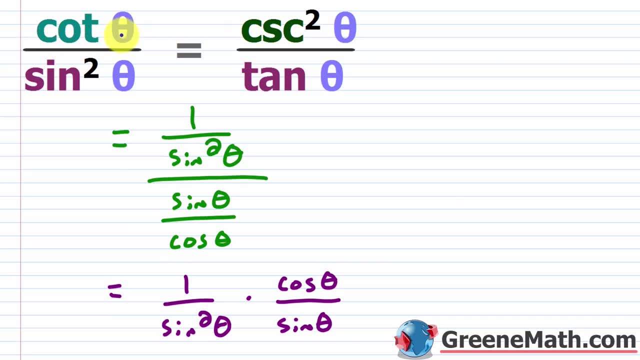 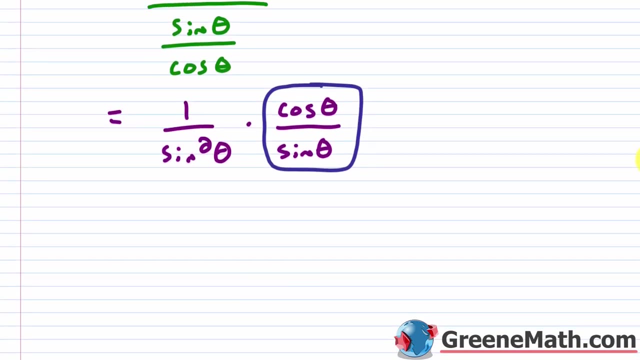 okay, Let's think about what we have. We have cotangent of theta over sine squared theta. Well, I have sine squared theta here, This right here, if you really think about your reciprocal identities, remember, cosine of theta over sine of theta is cotangent of theta, So I can replace that. okay, I can replace that. 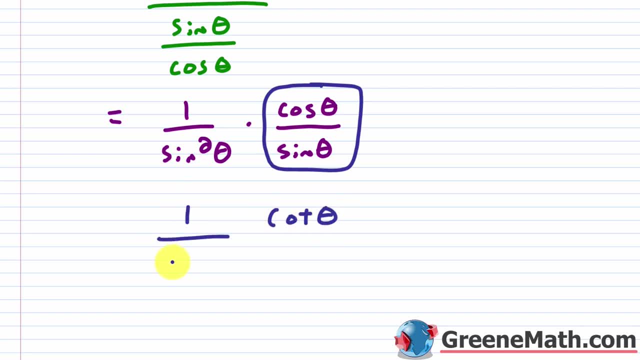 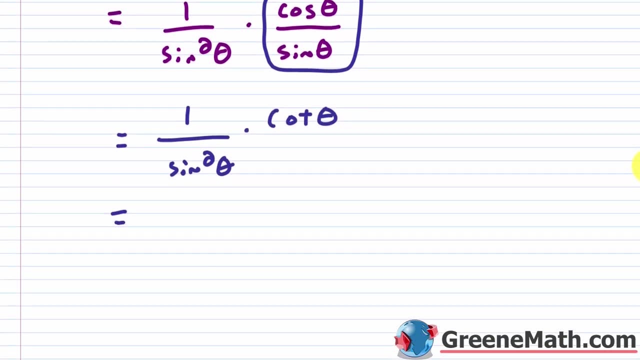 with cotangent of theta. okay. So I can put one over sine squared theta like this: multiply it by cotangent of theta, okay, And basically we're done right. All we have to do is multiply this through and say I have the cotangent of theta over sine squared theta. 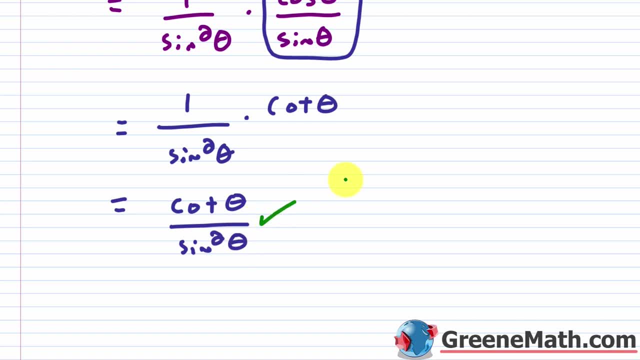 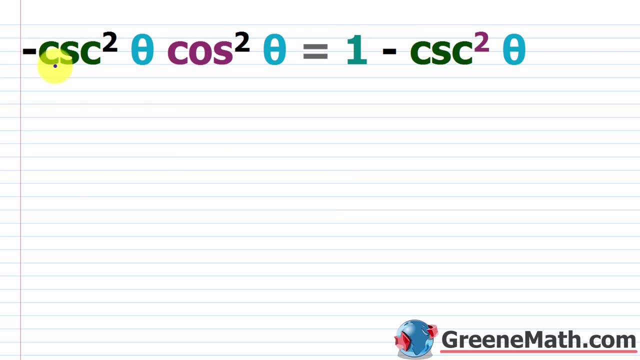 okay, So now you're left-sided and you're right-sided, you're right-sided, you're right-sided, so you put your checkmark there Again. just make sure you show your steps so your teacher can give you full credit. All right, for the next one, we have the negative. 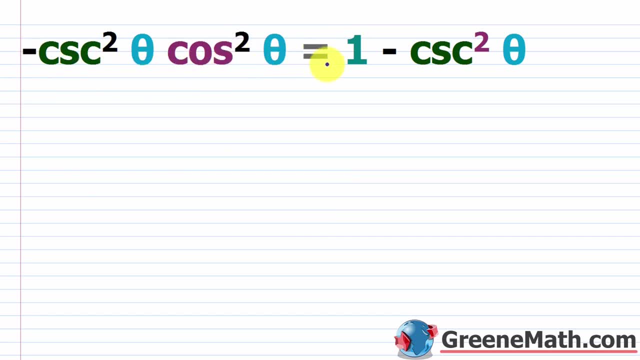 of cosecant squared theta times. cosine squared theta is equal to one minus cosecant squared theta. So for this guy you might be thinking that the right side is a bit more complicated. It looks kind of like the difference of squares right. So it is actually. You could factor that if you. 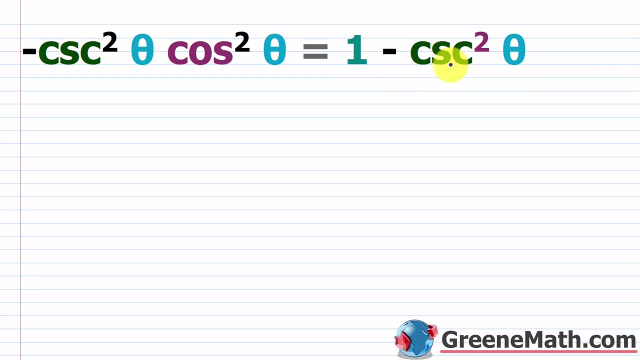 wanted to, but I'm not going to do that. I'm going to leave this side alone. Whenever I see something looks like this- I'm thinking about the Pythagorean identities- I have a minus or a plus with a one here, and this is squared. If I look at my little handout here, I want you to think about this one. 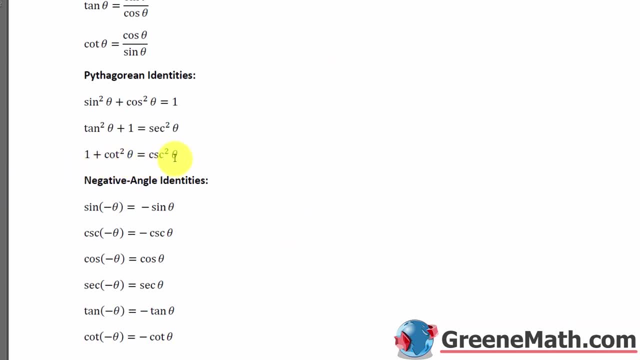 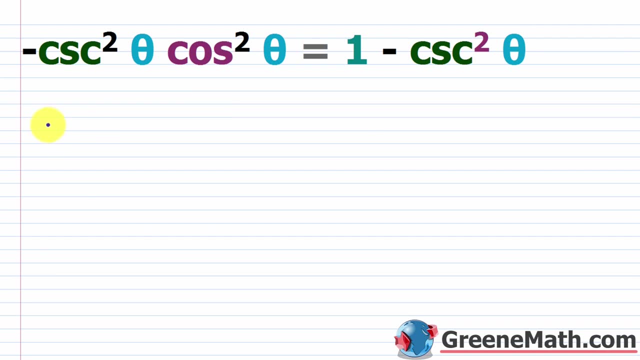 right here. So one plus cotangent squared theta is equal to cosecant squared theta, okay. So we'll come back to that in a moment and I'm just going to work through this. I'm going to flip the sides here. I'm going to put one minus cosecant squared theta- okay, is equal to. I'm going to put negative. 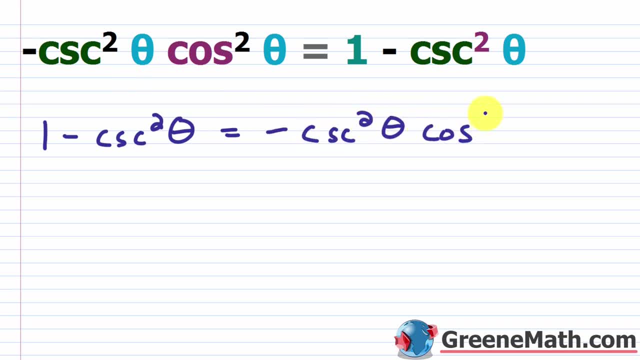 cosecant squared theta times the cosine squared theta. okay, So what I'm going to do first is just take this side right here and express it in terms of sine and cosine. Again, for a lot of these problems, that ends up being all you really need to do to end up with a solution. So I'm going to. 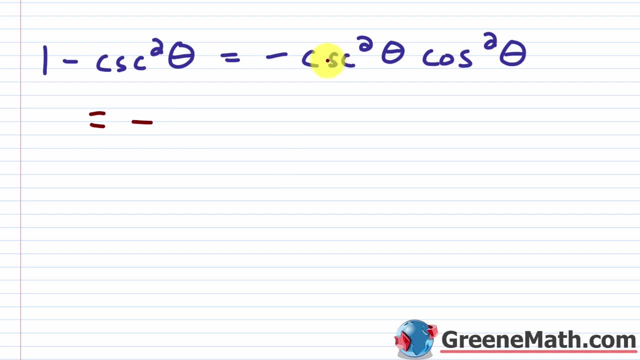 put equals over here. I'm going to change this. I'm going to put my negative out in front. Cosecant squared theta. again with the reciprocal identities, I can put one over sine squared theta. okay, This is times. cosine squared theta. 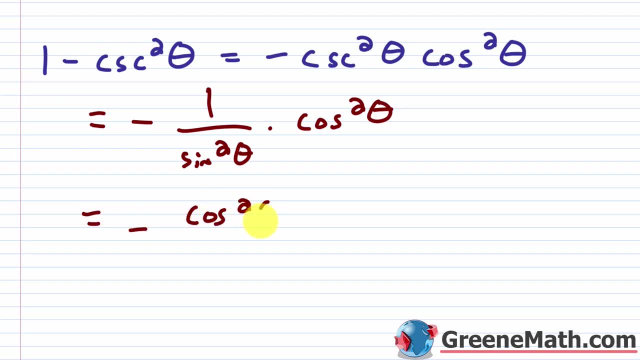 And then over here I have the negative of: I'll say: cosine squared theta over sine squared theta. Can I make a replacement here? Yes, because this guy right here is the cotangent of theta, right. So basically what I have. let me scroll down a little bit. 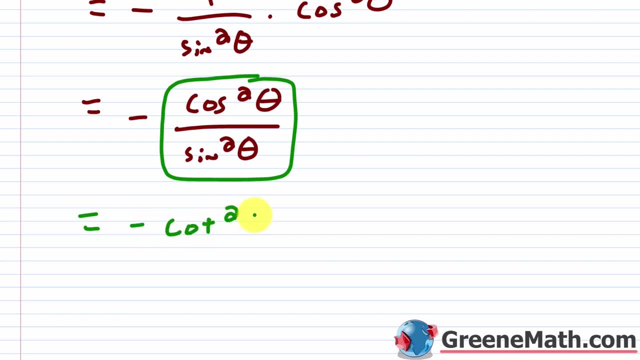 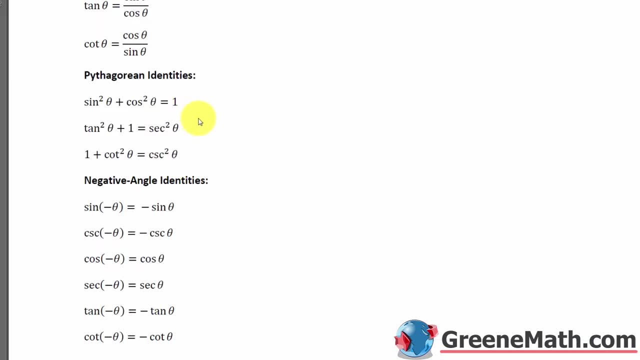 is the negative of the cotangent squared theta. Now, can I do anything with this? Remember I talked about this Pythagorean identity here. okay, Let's assume I moved this over here and this over here. So basically I would have one minus the cosecant squared of theta. 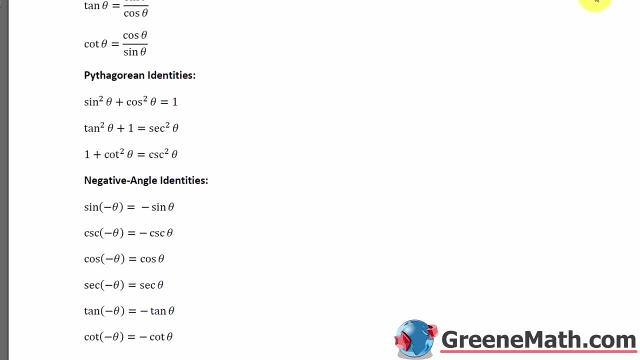 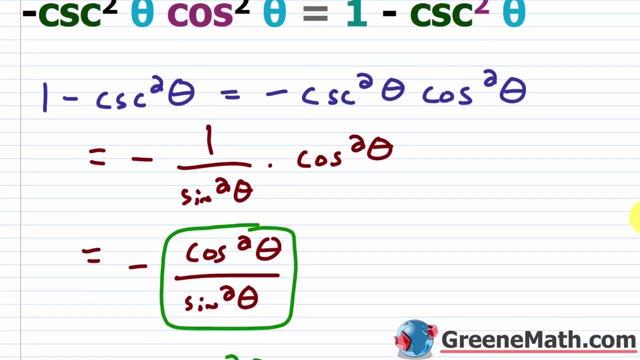 is equal to the negative of cotangent squared theta. So right now, I have the negative of cotangent squared theta and I can replace it with exactly this right here: one minus cosecant squared theta. okay, So that's what I'm going to do. So I'm going to say this guy right. 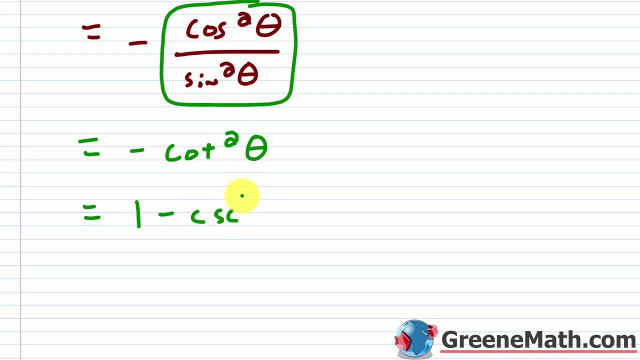 here is one minus the cosecant squared theta. okay, So now my left side exactly matches my right side. I'm going to put my checkmark there and I'm done. All right, let's take a look at a harder example. 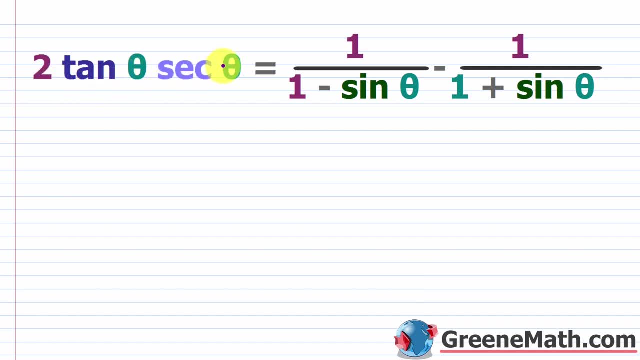 So here we have two times the tangent of theta, times the secant of theta is equal to one over one minus the sine of theta, minus one over one plus the sine of theta. So when you see this guy right here or this guy right here, you got to be thinking about conjugates, okay, So I'm definitely 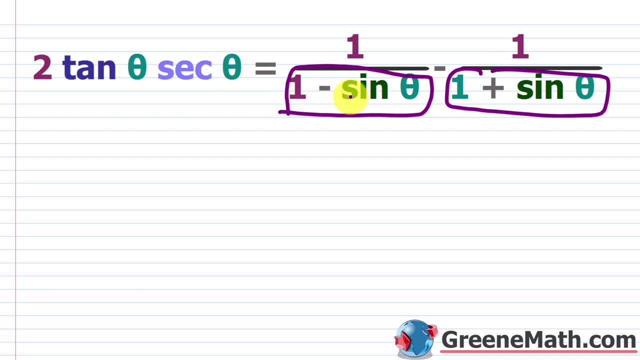 going to leave the left side alone and I'm just going to play with this right side Before I do anything. I just want to do this off to the side so I have a lot of room to work. I know that I would want to get a common denominator here, okay, So how would I do that Again? 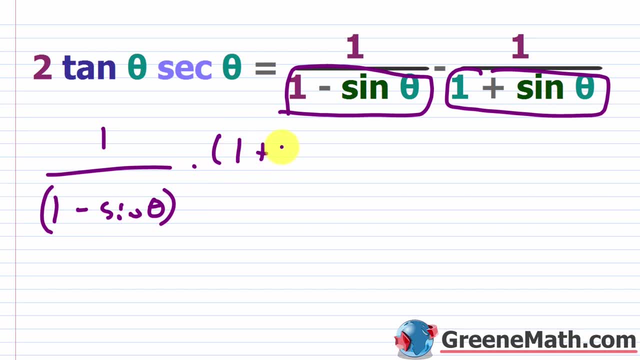 I'm thinking about conjugates. So here I would multiply by one plus the sine of theta. okay, Here one plus the sine of theta, to make that legal Again, this is one. I can multiply these together. So you see how this formula is going to work. if you had a minus b, that quantity times a. 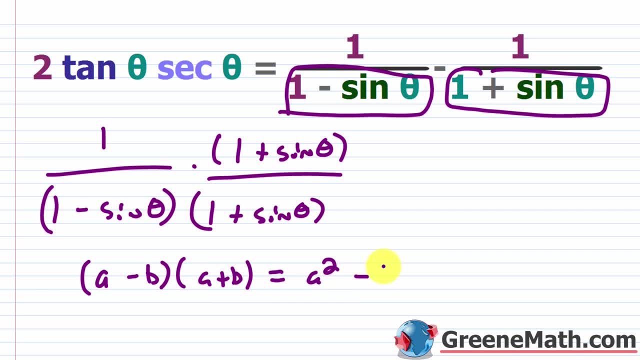 plus b, this quantity. Remember, this is a squared first guy squared, minus b squared minus the second guy squared. okay, In this case it's going to be no different. This is going to end up being one: the first guy squared. 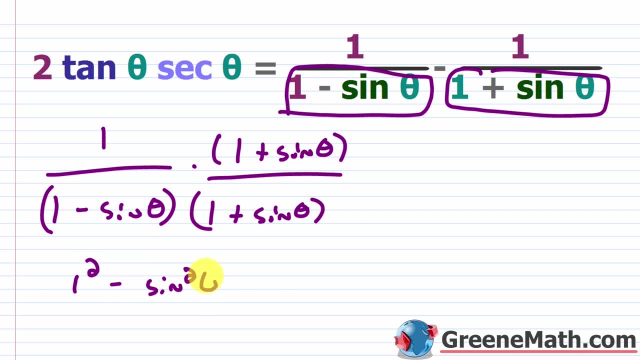 Then minus, you have sine squared theta. So sine squared theta. this second guy squared: okay. So up here, this would just be one, one plus sine of theta. okay, You can get rid of this. and then down here, this is going to be one. you don't need one squared minus the sine squared. 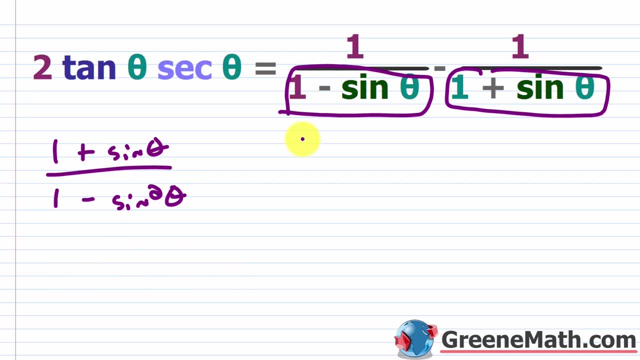 theta. okay, So that's going to be this part right here. For this part right here, I have a plus here. So basically, this part is going to be a minus. So I'm going to put a minus here and I'm. 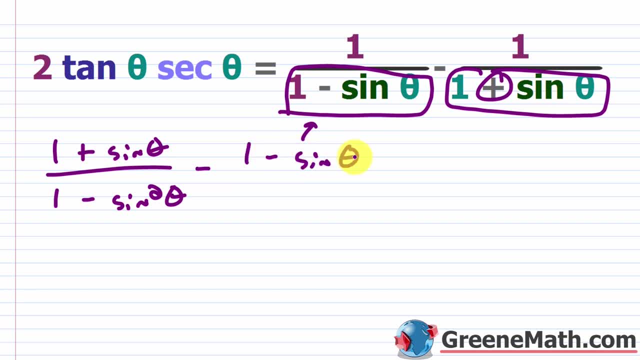 going to end up with what? One minus sine of theta in the numerator, because again, I'm going to multiply by one minus sine of theta here, one minus sine of theta here, and then down here. it's the same thing, right, It's the same thing. So it's going to be one minus sine squared theta, okay. 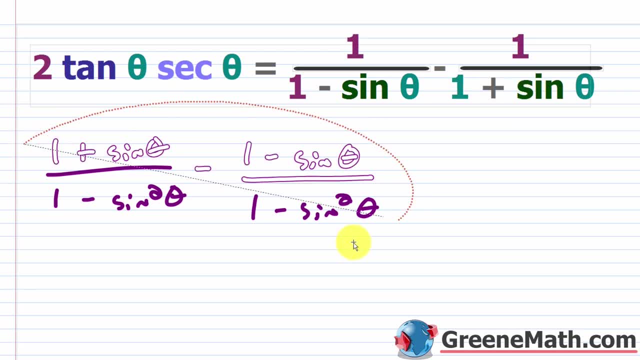 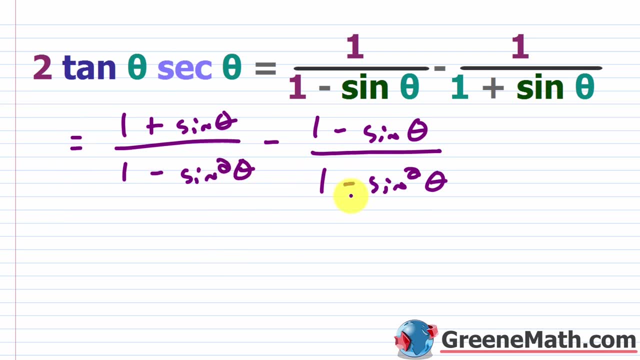 So let me erase this and let me slide this over so I get my formatting right. Slide this over just a little bit, put equals there And again I can write this with a common denominator, So you can even do this real quick right here. so we save a little bit of time and a little bit of effort. 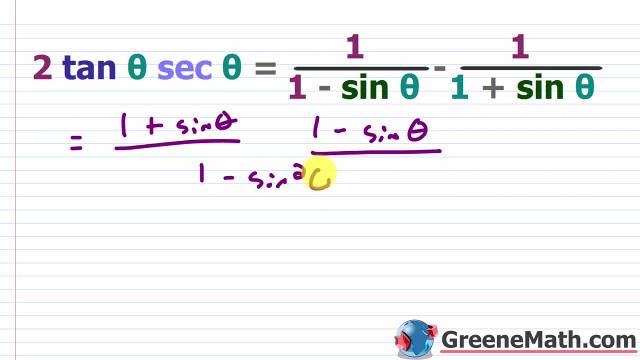 So let me just put one minus sine squared theta like this, and then I'll put this as one numerator with a minus here. But be very, very careful: When you're subtracting this away, you're subtracting away the whole thing. So go ahead and wrap that in parentheses to remind you that you need to. 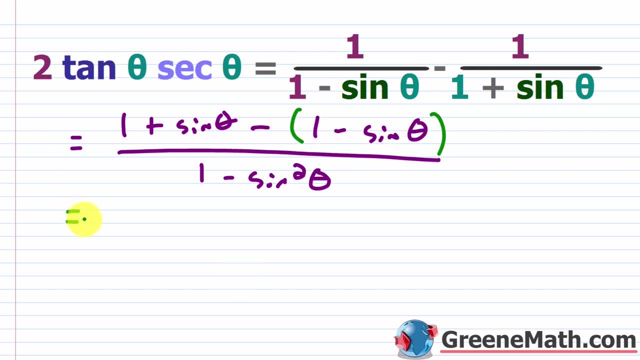 change your signs because you're subtracting the whole thing away. Okay, so let's keep going and see what's going to happen here. So I'm going to have one plus sine of theta. Again, you're going to have one minus sine squared theta over one minus sine squared theta. So what can we do? 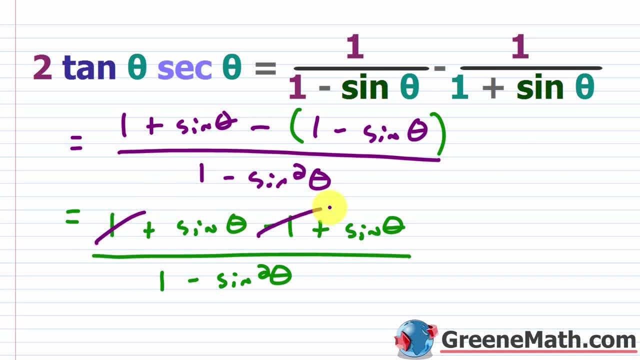 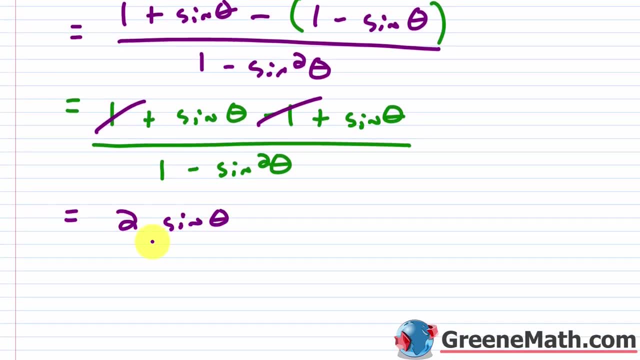 here. Well, we see immediately that this is going to cancel. okay, So now I basically have two times sine of theta. So two times sine of theta over one minus sine squared theta. Now remember in the hints we saw that one minus sine squared theta was cosine squared theta. Again, if you go back to 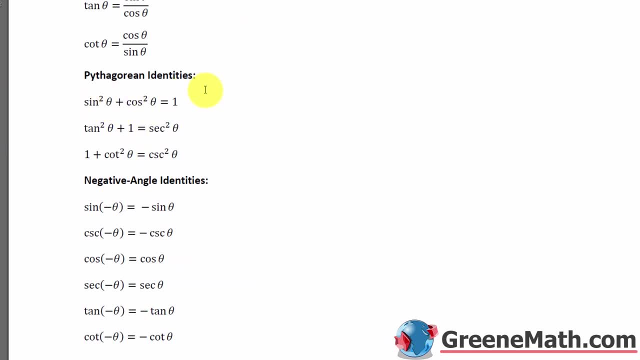 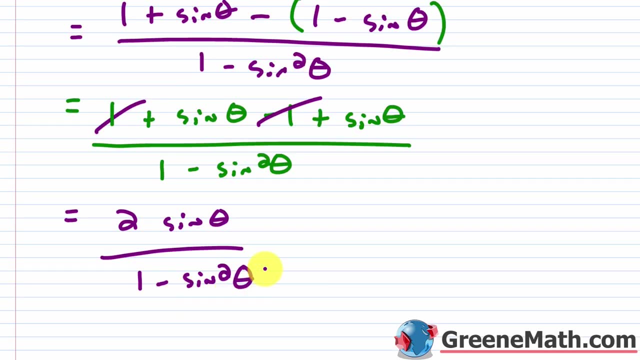 this: if you have this guy right here and you just subtract this away, so one minus sine squared of theta would give you cosine squared theta. So if we come back here, I can replace this with cosine squared theta. So let's go ahead and do that. So I'm going to put equals two times sine. 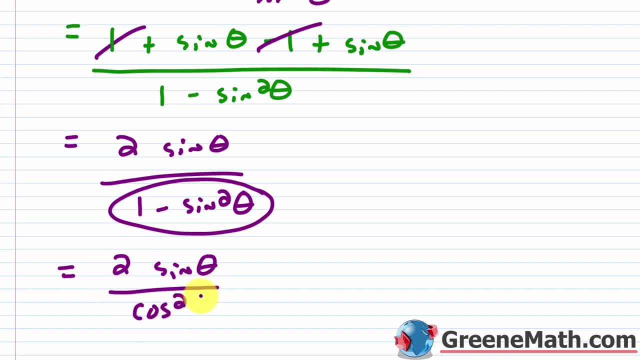 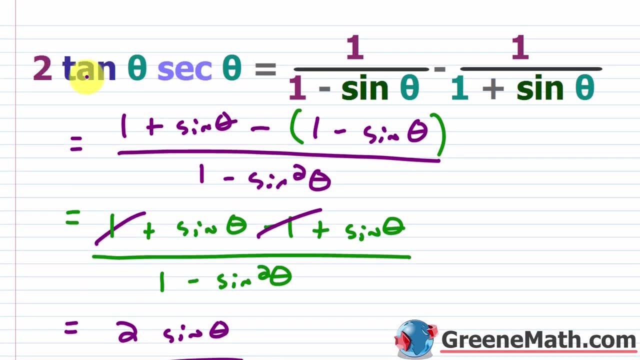 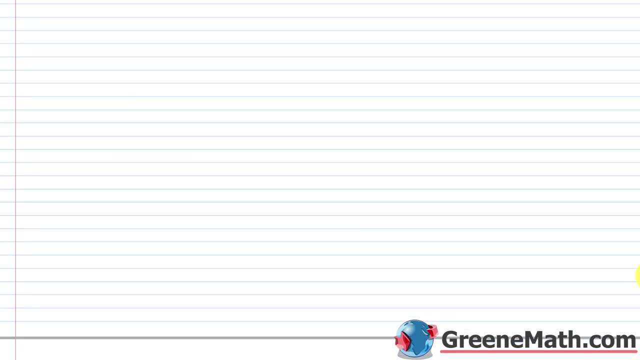 of theta over the cosine squared theta. okay, Now is this getting close to what we want? Let's go back up and see where we are. We have two times the tangent of theta, times the secant of theta. So are we close to that? Well, I see I have the two. I need the tangent of theta and the secant. 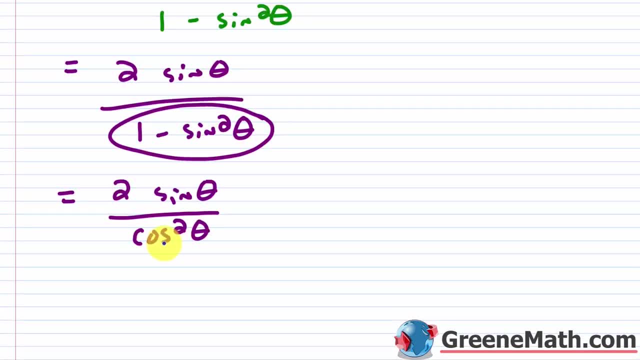 of theta. So to get this, I'm going to break this up. Remember: cosine squared theta can be written as cosine of theta, times cosine of theta. okay, It's just this times. this gives me cosine squared theta. Now, up here I have two times sine of theta. Now think about it. If I have sine of. 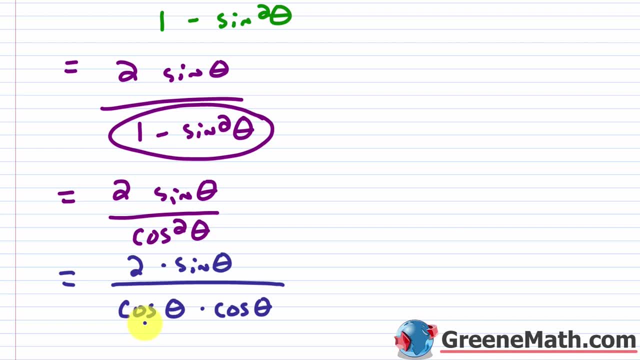 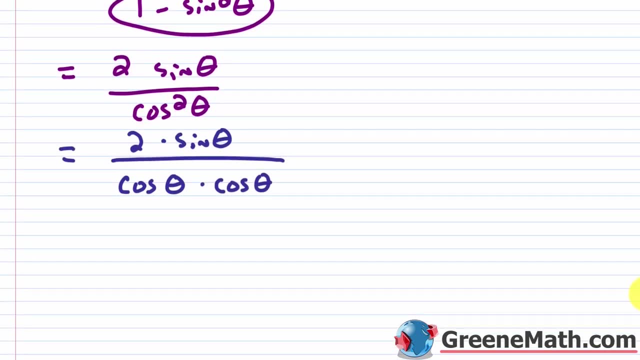 theta over cosine of theta, that's the tangent of theta, okay. And if I have one over cosine of theta, that's the tangent of theta. So I already have what I need, okay. You just need to break things up so you realize what's going on. So I'm going to put this as two times sine of theta over cosine. 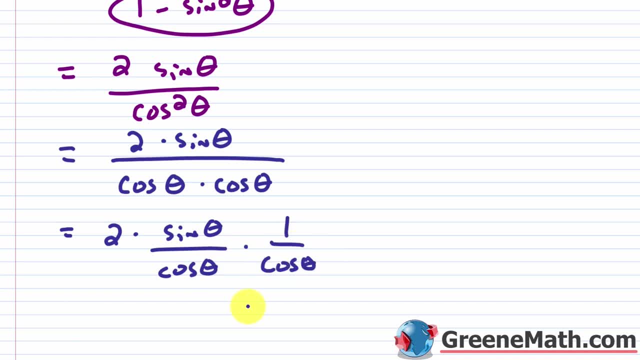 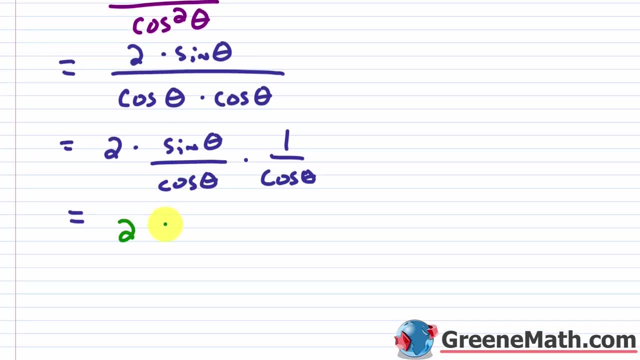 of theta times, one over cosine of theta, And then I'm just going to again replace this with what I'm looking for. So in this particular case, it's going to be what? Two times? this is going to be the tangent of theta times. in this case, this is going to be the secant of theta And now the left. 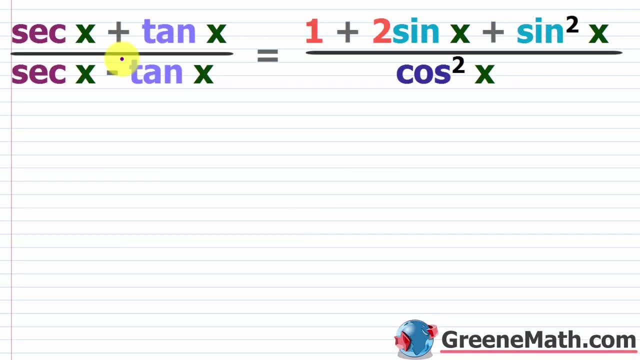 side of theta is going to be the tangent of theta, So I'm going to go ahead and put my check mark there And again, I'm done. All right, let's take a look at one final problem. And this guy is going. 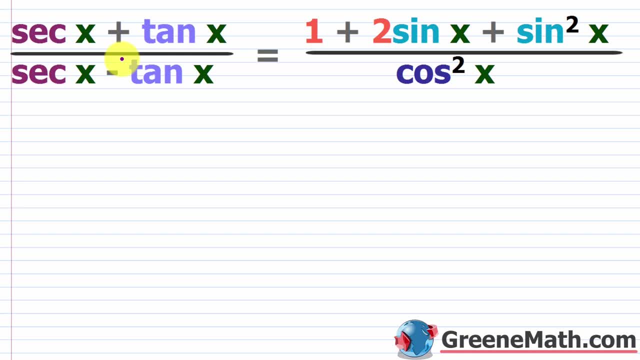 to be pretty challenging overall. So I encourage you to pause the video and try this on your own, But before you do so, I want to just give you a little hint that you basically want to get both of these to a common expression. okay, So you want to work on one side, get it down to in terms of sine. 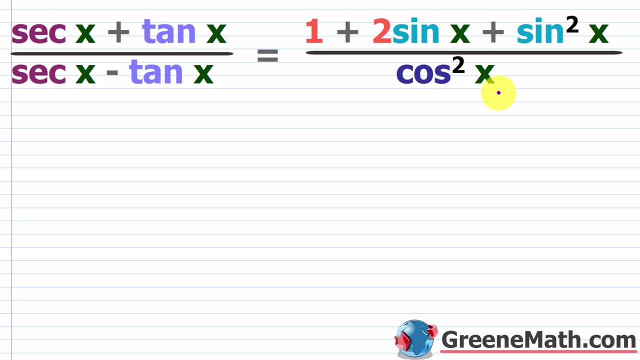 and cosine. This side is pretty hard. If you are not used to working with these. this side's pretty hard. So I'm going to pause the video and try it- And hopefully you did give that a try- And I'm just going to start with the left hand side here. okay, So I'm going to start by just taking this guy. 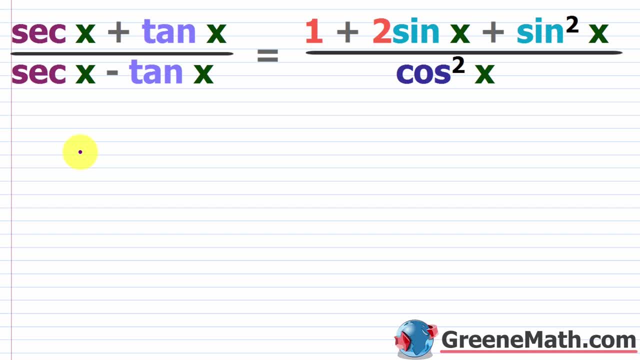 and trying to write it in terms of sine and cosine. So how can I do that? Let's start out by just putting that we're working on the left hand side. okay, Some teachers want you to do this, others don't care, So just get with your teacher And I'm going to first copy the left hand side. 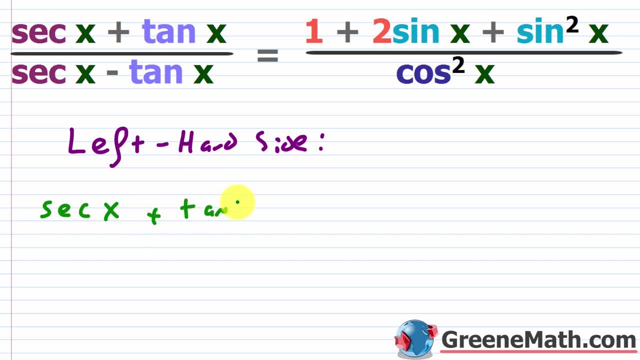 So I have the secant of x plus the tangent of x over the secant of theta. So I'm going to do that. So I'm going to do that, So I'm going to do that, So I'm going to of x minus the tangent of x. Now, lots of ways to do this. I'm going to go through one, that is: 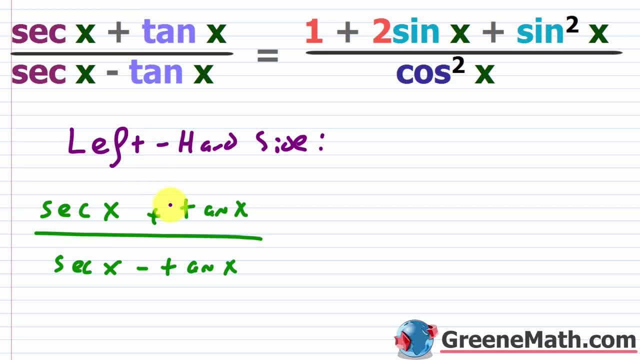 probably not obvious If you haven't worked a lot of these problems. Remember: the secant of x, by definition, is equal to one over the cosine of x. okay, So if I multiplied this secant of x, which is one over the cosine of x times the cosine of x, I would get one. okay, So in other 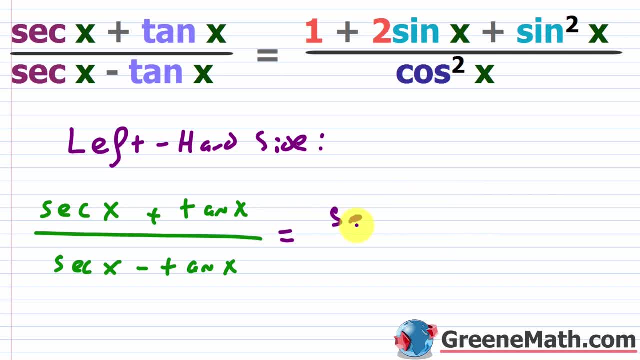 words if I did this guy right here. let me just copy this real quick: So: secant of x plus the tangent of x over the secant of x, minus the tangent of x. If I multiply this guy by the cosine of x over the cosine of x, when I distribute this here this is going to be one. 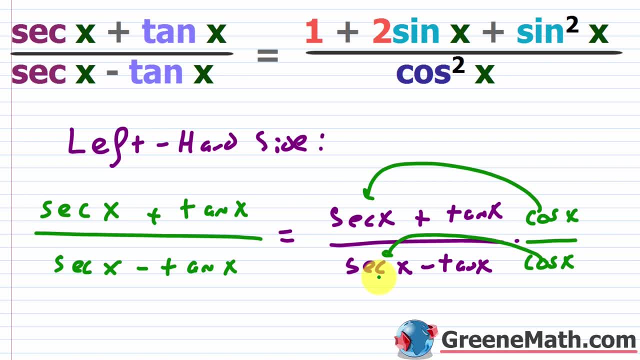 When I distribute this here, this is going to be one. Another benefit is when I distribute this here and this here. think about the fact that the tangent of x is the sine of x over the cosine of x, So the cosine of x is going to cancel in each case. So I'm going to end up. 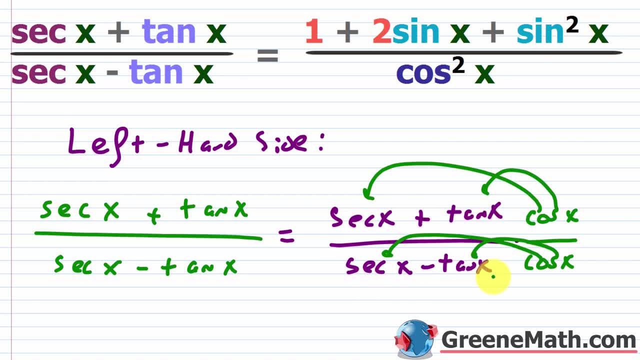 I'm going to end up with one plus the sine of x and one minus the sine of x. So that's pretty simple, okay? So that's how I'm choosing to do this. Again, you could arrive at this a different way. 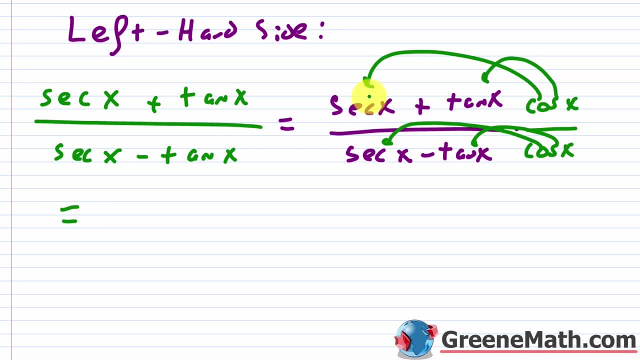 So let me just put equals over here. This multiplied by this is going to give me one, okay, And then plus, let me just write this out: So the tangent of x times the cosine of x- we know we can cancel that further, And then we have again cosine of x times secant of x is one. 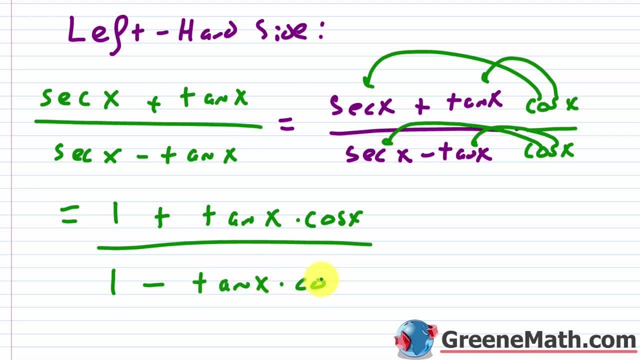 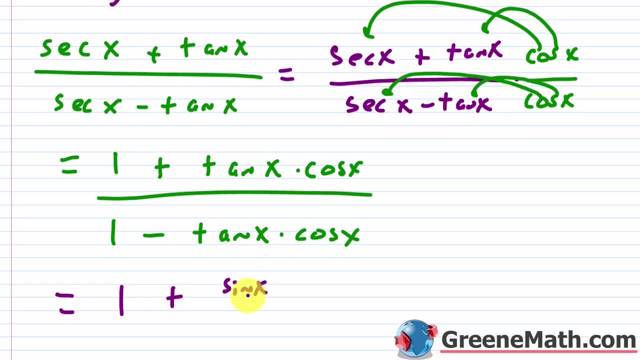 minus, we'll have the tangent of x times the cosine of x. okay, So that's pretty simple. So from here I'm going to again keep simplifying. Let's put one plus. I'm going to do sine of x over cosine of x times the cosine of x. Again, this is going to cancel. So this cancels. 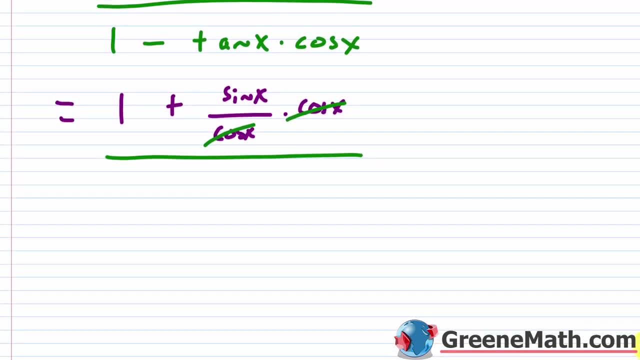 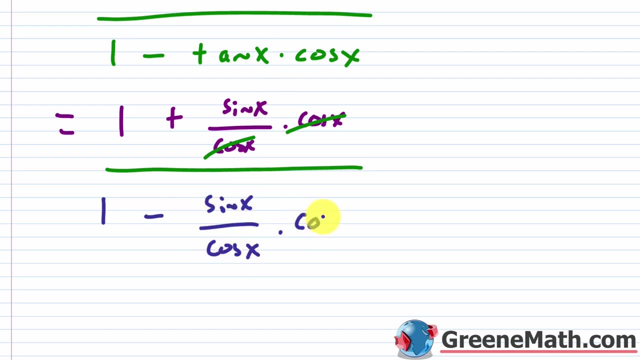 with this And this is over. Let me get some more room here. I think I'm going to run out, So we have one minus again. I'm going to write this as the sine of x over the cosine of x times the cosine of x. okay, So this is going to cancel and I have the sine of x there, okay. 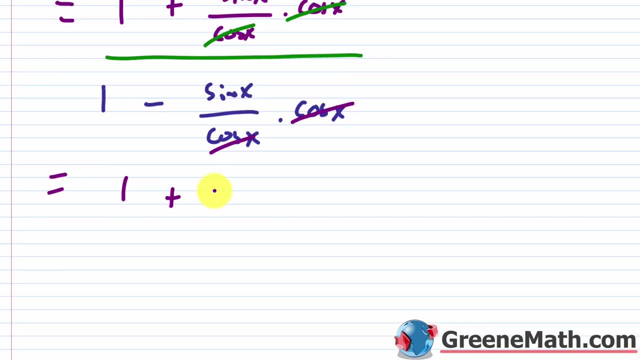 So let's just write this one more time. We'll put one plus the sine of x over one minus the sine of x. So that's pretty simple. It's in terms of sine, okay, And basically now what I want to do is try to get the right-hand side to match this. 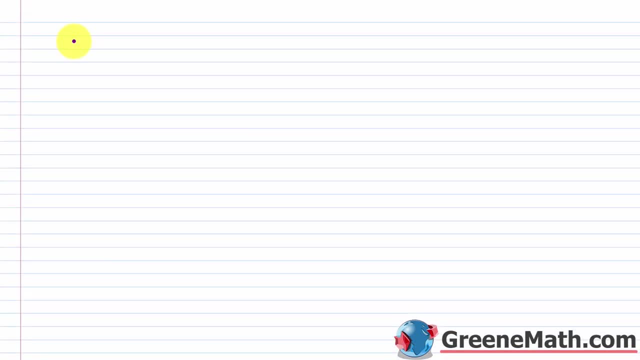 and you're going to find that that's pretty simple. So let me start a new sheet here and I'm going to say the right-hand side, okay, And let me make that a little bit better. So let me put the right, and I'm going to try carefully to write this So right-hand. 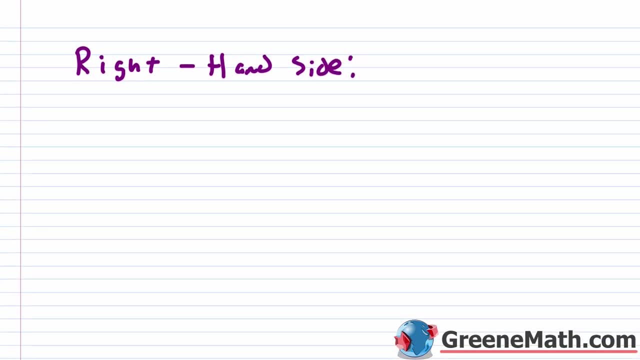 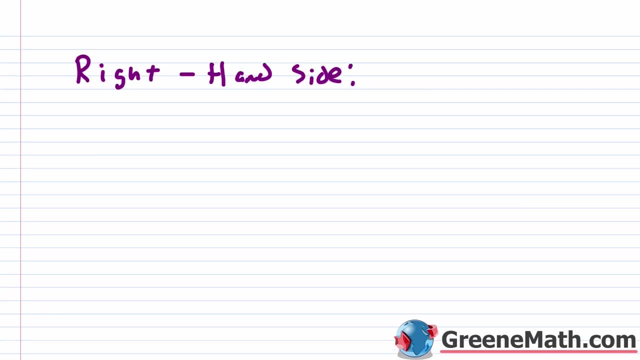 side. okay, Penmanship is hard for me. So let's come back up and let's think about this, guys. So we have one plus two times the sine of x plus sine squared of x over cosine squared of x. So let's come down. So we have one plus two times the sine of x plus sine squared of x, okay, over. 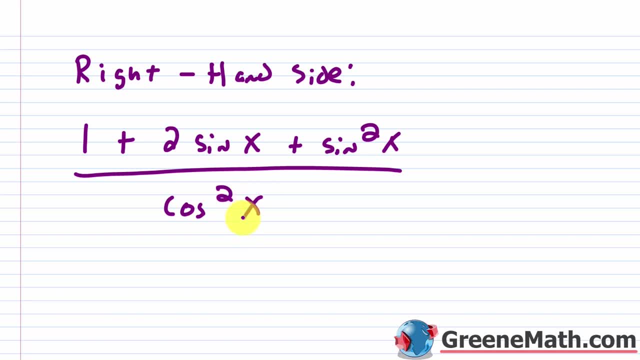 we're going to have the cosine squared of x. So the first thing is you should be thinking about factoring when you see this pattern Again. this is basically where you have x plus y quantity squared right, It becomes x squared. so first guy squared plus two times. 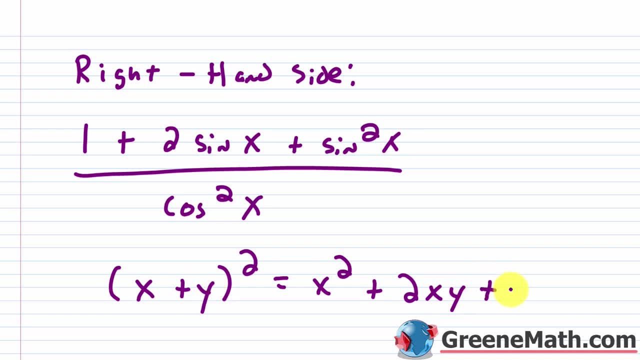 the first guy times the second guy, so two times xy plus the last guy squared. okay, That is exactly the pattern you have here. This is going to be basically one plus sine, okay, of x, quantity squared. So I'm going to take this guy and let me do this properly. So let me just kind of slide. 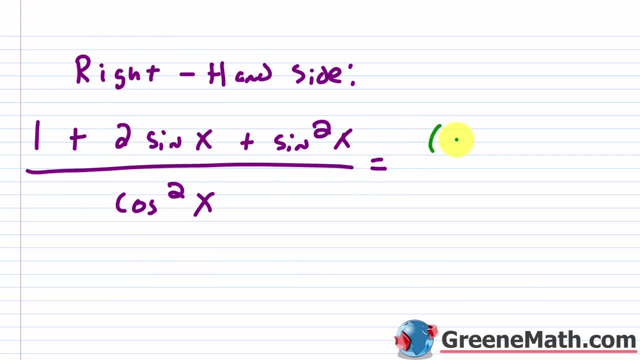 this down a little bit. okay, I'm going to put equals. So I'm just going to say: this is one plus the sine of x, quantity squared. So I'm going to put equals. so I'm just going to say: this is one plus sine squared over your cosine, squared of x. okay, So I'm going to put equals over here. 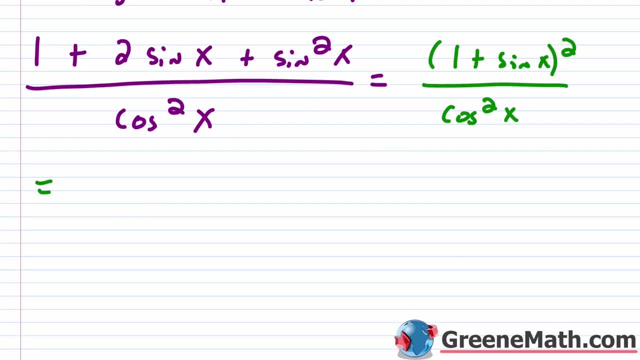 So what am I going to do with this, now that I've factored it Well again, if you see something like cosine squared of x and you see something in terms of sine of x, I want you to think about the fact that this can be replaced with one minus sine squared of x. okay, So I'm going to write. 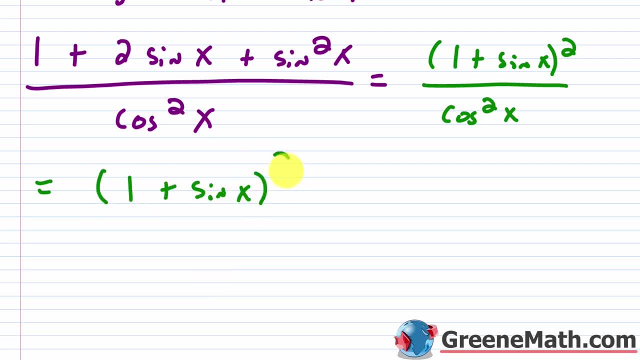 this as one plus sine of x quantity squared over. this is going to be one minus sine squared of x. So at this point some of you are thinking that there's something weird going on. this doesn't match this, but it will in a second. This is the difference of squares, so you need another. 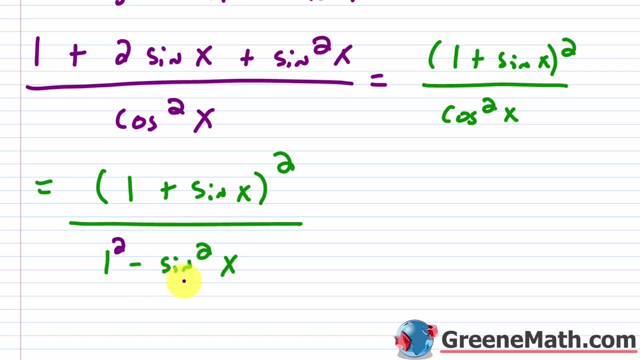 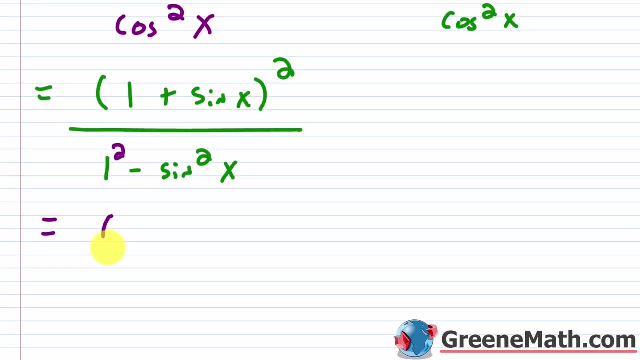 factoring pattern here. This is one squared, basically minus sine squared x. So I'm going to rewrite this and then it's going to be completely obvious what's going on. okay, So first let's go ahead and write this as one plus sine of x times one plus sine of x. okay, So I'm? 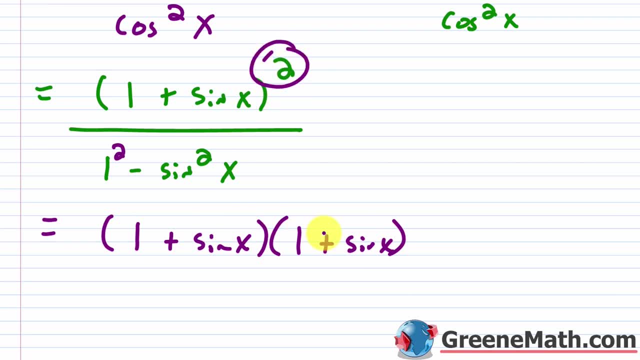 just expanding this. Nothing illegal about that. I have an exponent of two there, so I'm allowed to do it. okay? Then down here I'm going to factor this as one plus sine of x times one minus sine of x, and now it is completely clear what I'm doing, okay? So this: 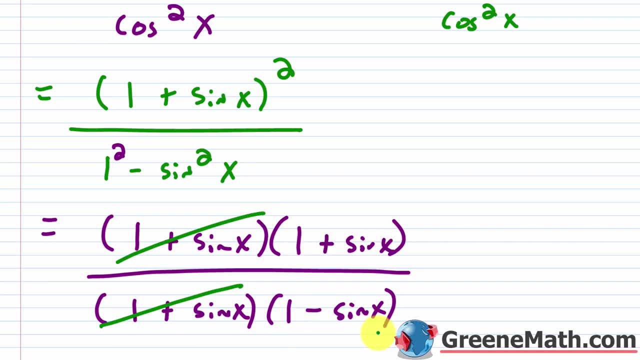 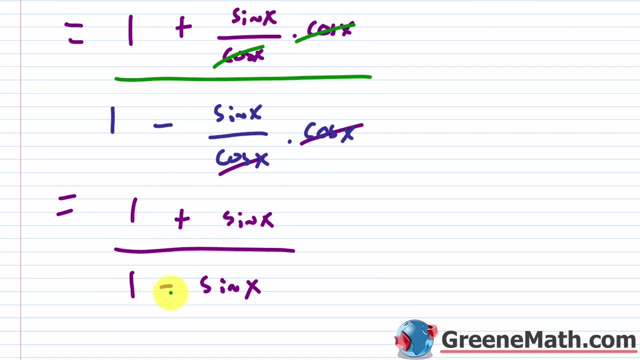 cancels with this and I have one plus sine of x over one minus sine of x. Again, if we go back, what did we have here for our left-hand side when we worked it? One plus sine of x over one minus sine of x. So what I'm going to do here, I'll just put equals: one plus sine of x. 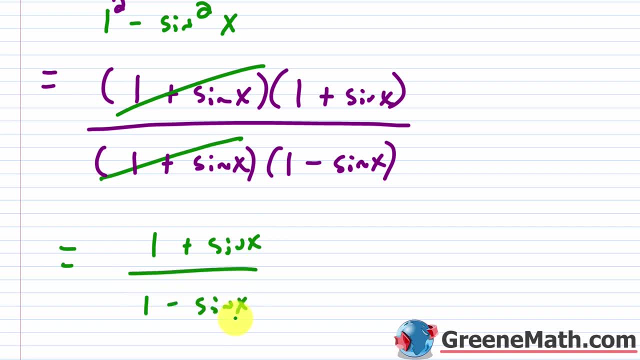 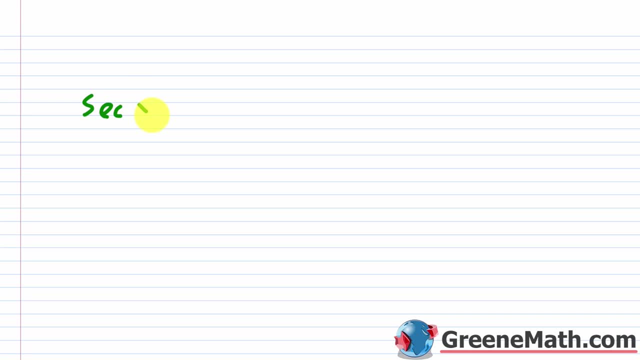 over one minus sine of x. and to complete this guy, you might just want to write your basically three expressions here. So I'm going to say that the secant of x plus the tangent of x, so plus the tangent of x over, and I don't know if I can fit this all on the screen. 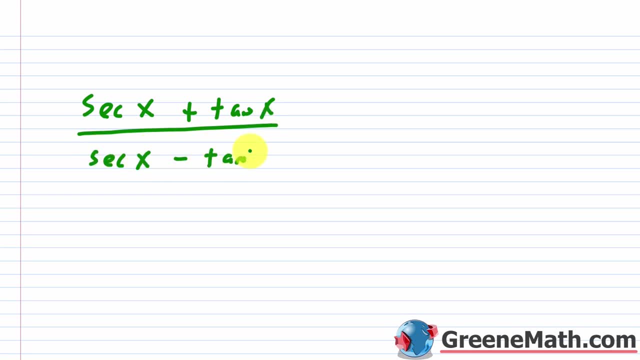 but I'm going to try. So the secant of x minus the tangent of x- let me scroll this down, I'm going to try to write: smaller- is equal to. we have this one plus the sine of x over one minus sine of x. and to complete this guy, you might just want to write your. 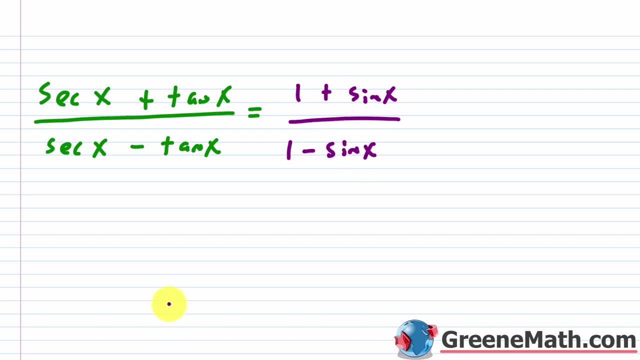 over one minus the sine of x. So this is what we found from working the left side and the right side. okay, So this is your, basically your common third expression. okay, And this is going to be your one plus your two times sine of x plus sine squared of x. Let me see if I can scooch this. 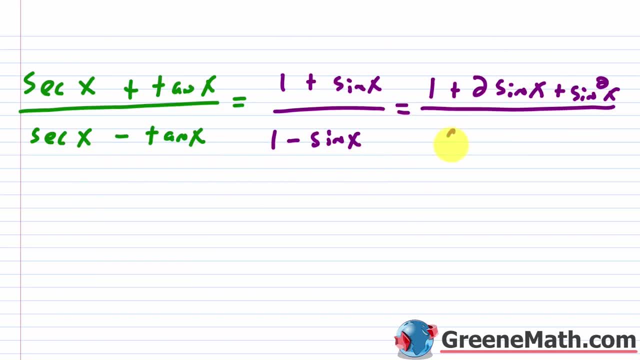 down just a little bit more And then over you had your cosine squared of x. okay, So this is going to basically do it for this guy. Again, you're not going to put the sine of x over one minus the tangent of x, okay, So you're going to put the sine of x plus the tangent of x, squared of x. 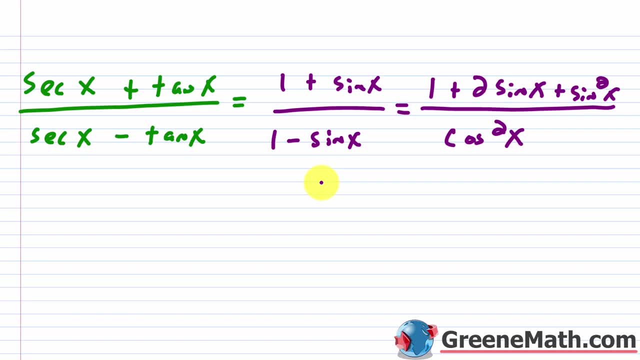 okay. So this is going to be your one plus your two times sine squared of x. okay, And this is going to be your one plus your two times sine squared of x. squared of x. squared of x. Let me show you how to do this, So you're going to probably see too many of these if you're on a basic test. 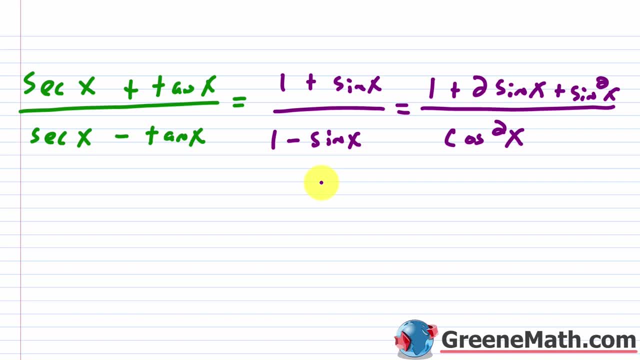 you're probably going to get maybe one of them towards the end. They realize how much time these guys take. okay, So if you get something where you're just working and working and working on one side you can't get anywhere, go ahead and get it in terms of sine or cosine, stop. 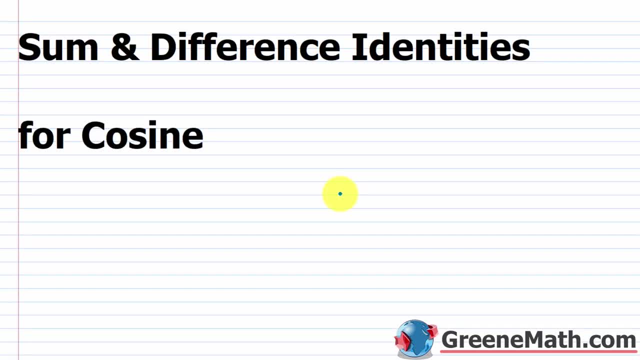 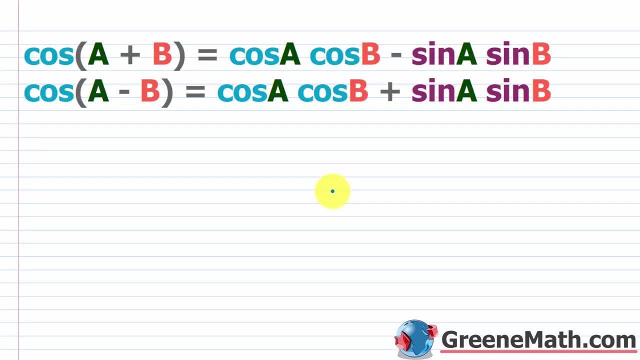 and then start working the other side. See if you can get it to match. In this lesson we want to talk about the sum and difference identities for cosine. All right, so let's start sum identity for cosine. So let's say you had the cosine of some angle a plus some other angle b. 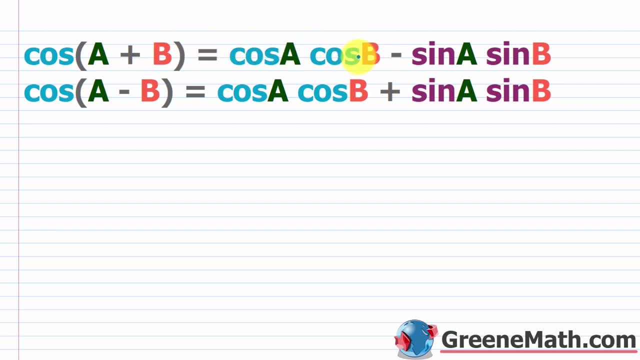 This is equal to the cosine of a times the cosine of b, minus the sine of a times the sine of b. So let me give you a quick example. We're going to work on examples like this in a little while, but just so you see what's going on. let's say you had the cosine of, let's say, 45 degrees plus. 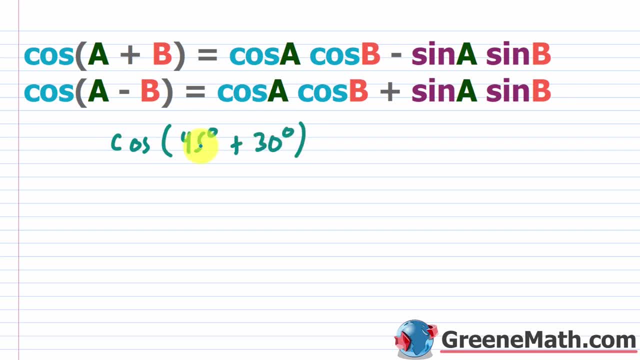 30 degrees. So we know this is the same as if you added those two angles and you said you wanted the cosine of 75 degrees. But you can break this up if you wanted to get an exact value. I'll talk more about that in a 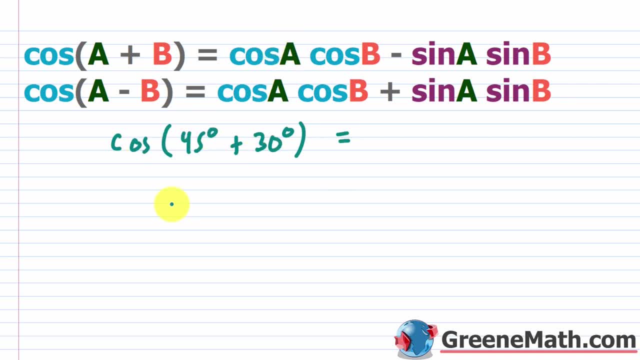 little while. But basically, if you wanted to do this, it's the cosine of the first guy, so the cosine of 45 degrees, then times the cosine of the second guy, so times the cosine of 30 degrees, then minus the sine of the first guy, so the sine of 45 degrees, and then times the sine of the last. 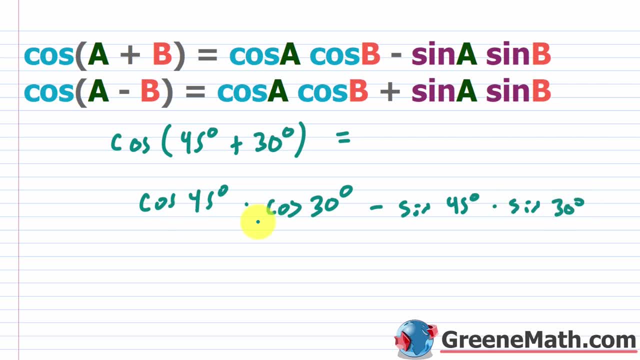 guy, or the second guy, which is 30 degrees. So this is how you would have to set this up. A lot of times you're going to have the cosine of 45 degrees plus the cosine of 30 degrees. That does not work, Okay, so you can't do that. You have to use this formula. Now for the other guy, let's say: 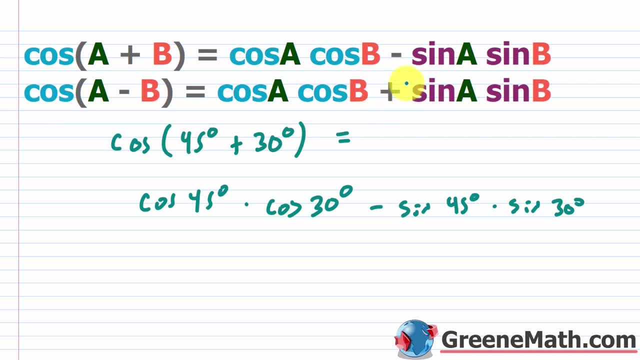 you have the cosine of a minus b. what's going to change is the sine here. So I always remember this is the opposite: sine: cosine of a times cosine of b, now plus sine of a times sine of b. So, for example, if you did the cosine of 45 degrees minus 30 degrees, well, now I'm looking for the 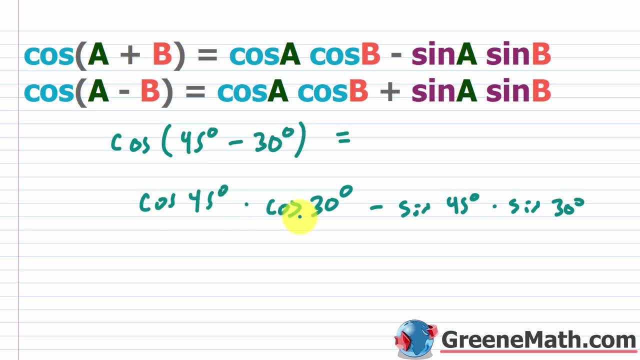 cosine of 15 degrees, and it's still cosine of 45 degrees times cosine of 30 degrees. This is now plus the sine of 45 degrees times the sine of 30 degrees, So it's just a change in the sign. So 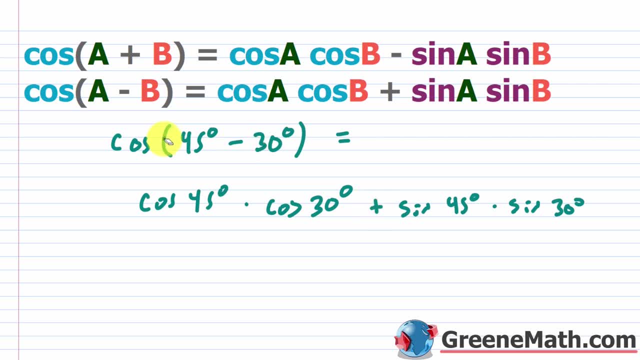 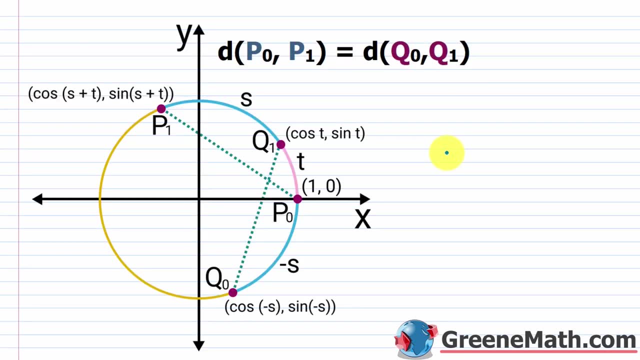 this sign, and this sign will always be different. Now let me get rid of this And let's talk about where this guy comes from. What you'd want to do is draw yourself a little unit circle on a piece of paper, And so again, this point right here. we know the x coordinate would be one and the y 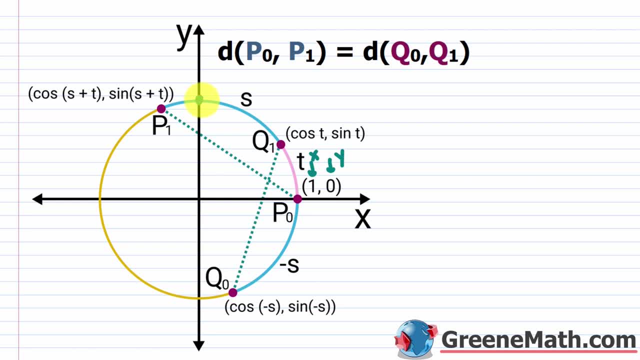 coordinate would be zero. Again, we're on the unit circle. If you went around and labeled these points zero comma one, then this point right here would be negative one comma zero, And then lastly, this point down here, this would be zero comma negative one. So again, we're on the unit circle. So we know. 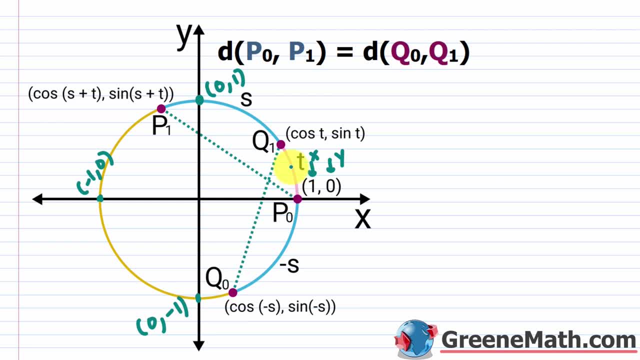 if we're on the unit circle and let's say starting here and going to here, I have this arc with length t. well then, I know the coordinates for this point q, sub one. the x value is the cosine of t and the y value is the sine of t. Now, if I keep going and let's say I end up at this point, right. 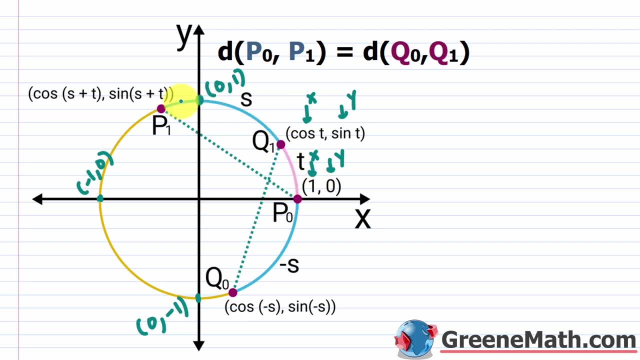 here. well, now I have an arc that has a length of t plus s, or you could say s plus t. So the x value here for this point is the cosine of s plus t, And the y value here is the sine of s plus t. And then 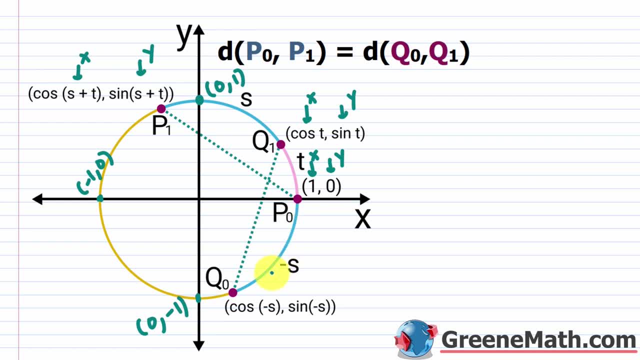 if I come this way, notice that I'm rotating clockwise. So here I would say: this is negative s. So whatever this is right, here it's the negative of that. And so if I look at this point, q sub zero, the x value here is the cosine of negative s And the y value here is the sine. 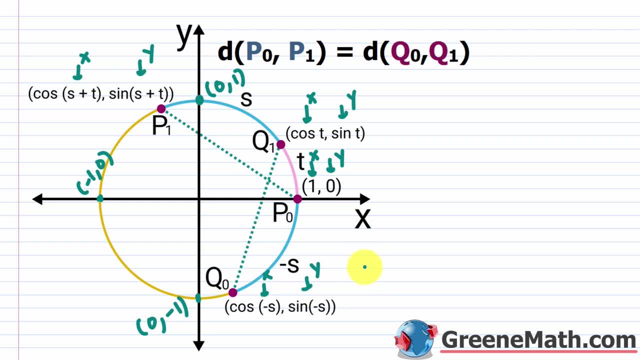 of negative s. Now, using the negative angle identities, you can really say that this is the cosine of s, because the cosine of negative theta is the same thing as the cosine of theta. And then you can say that this is the negative of the sine of s Because, again, if you have the 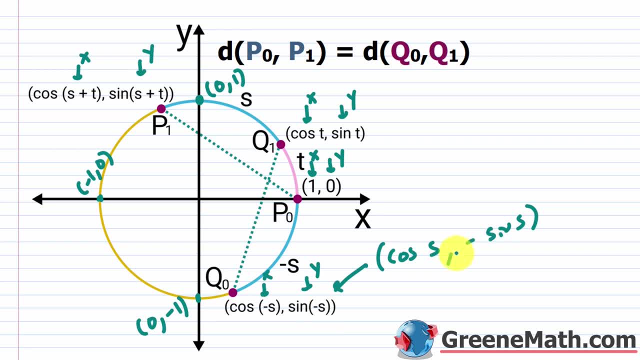 sine of negative theta. it's equal to the negative of the sine of theta, So we're going to be using this right here instead of this right here. Alright, so we have that settled, And now what we want to move into is we want to identify that we have these two. 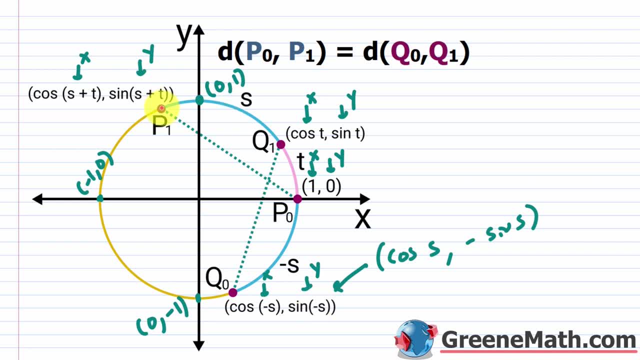 two equal arcs. So hopefully you can see this, the arc length. if I think about here to here, so this has s and it has t, would be the same as if I consider: let me change my color here from here to here. right, Forget about the fact that this is negative s Again. this guy and this. 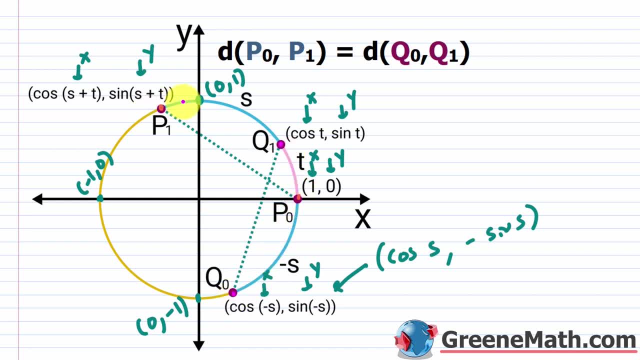 guy. in terms of the arc length, it's going to be the same. So you have s plus t, and here you have s plus t. So let me draw this out so that nobody's lost, And probably I should change the color again. Let me use this like red here. So let me trace this as good as I can, And then I'm going to 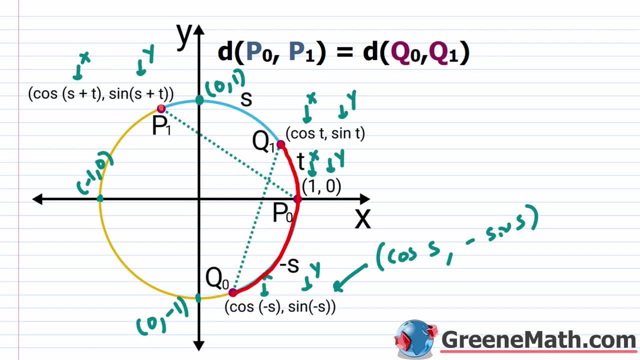 trace this as good as I can. So this arc here would be equal to this arc here, And I'm going to go underneath a little bit like that. Okay, so we can see that those two arcs are equal. And when you have equal arcs, they are what we call subtended by equal chords. So this chord here, 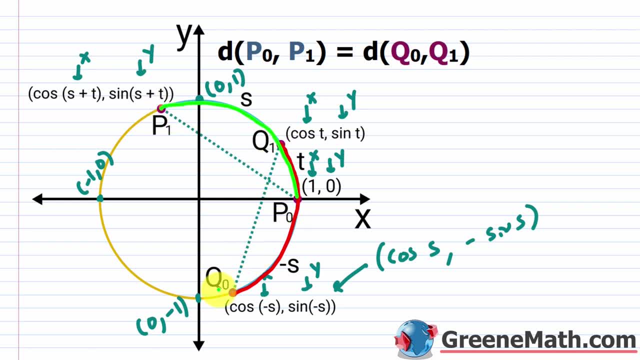 and this chord here. these two are going to be equal, right. So you see, up here I've written that the distance from P sub zero to P sub one- so that's this right here- is equal to the distance from Q sub zero to Q sub one. So this is going to be equal to this arc here and this arc here. 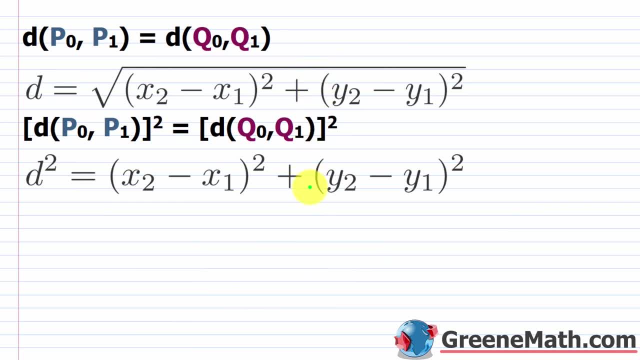 q, sub 1.. Okay, so that's this distance right here. So I went ahead and already set everything up for us. So what you would want to do from this point is write out your distance formula. Remember, we're on a coordinate plane And if we want to find the distance between two points, we say the. 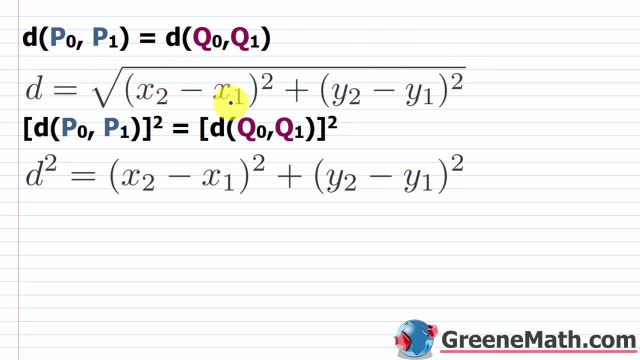 distance is equal to the square root of. you have x sub 2 minus x sub 1 quantity squared, plus y sub 2 minus y sub 1 quantity squared. Now what I did was I went ahead and squared both sides of this. 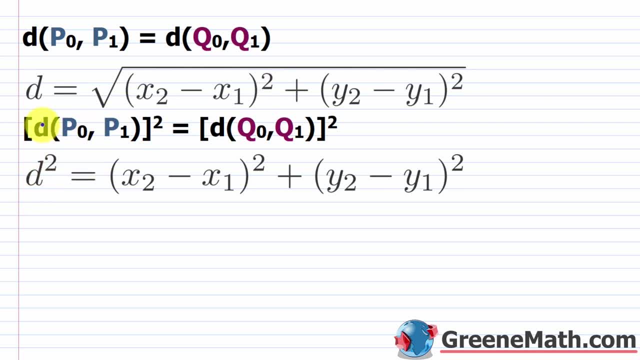 So I'm working with the distance squared now. So I'm saying the distance between the point p sub 0 and p sub 1, that guy squared- is equal to the distance between the point q sub 0 and q sub 1, that guy squared. So what we're going to do is just work on one side at a time And then I'm 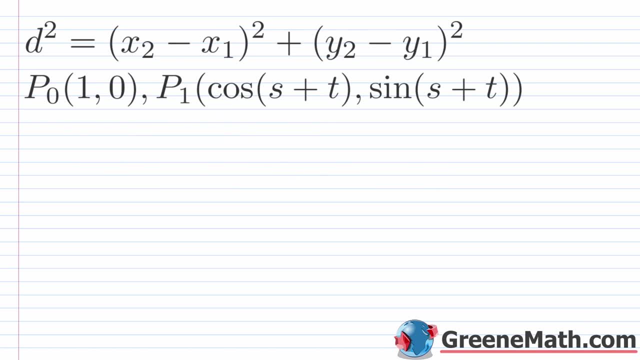 going to set these two guys equal to each other And you'll see, you have your formula. So, first off, I have again the distance squared here And I have my two points. So let me write this out. I'm not going to write: the distance squared equals, we don't even need that, I'm just going. 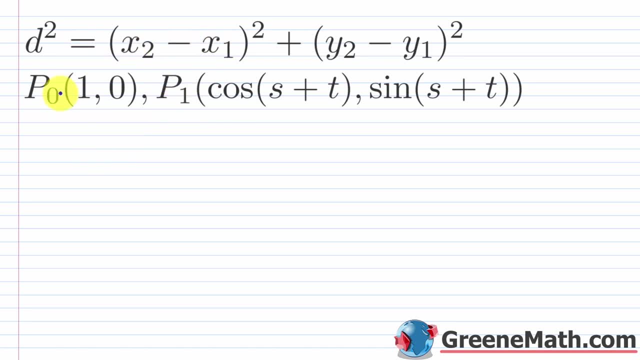 to plug in here. So I'm going to consider p sub 1 as my second point and p sub 0 as my first point. So let me get the x coordinate here. So this would be the cosine of this: s plus t, And then this guy right here would be minus. you would want your one here. 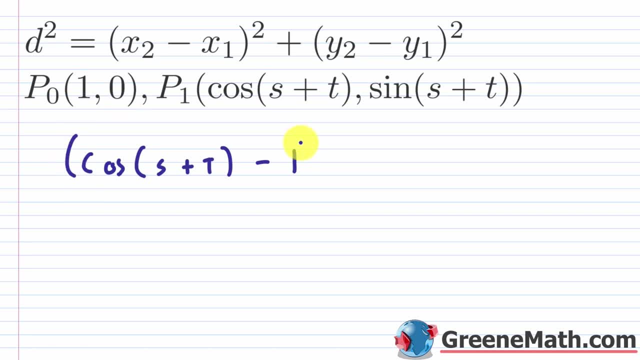 Okay, so I took the x coordinate here and the x coordinate here. Let me wrap that and square it. then we have plus. So now I'm working with the y's, So the y from the second guy here. so that's going to be your sine of this s plus t, And then we would have minus. 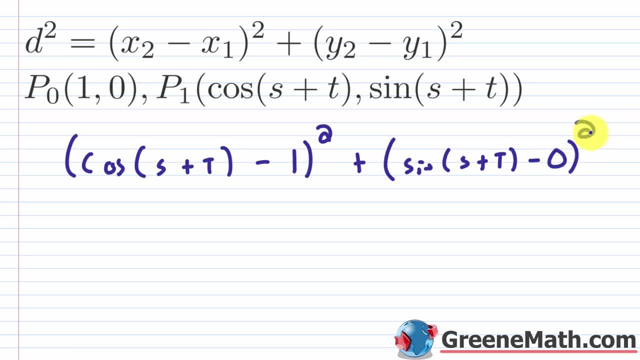 your y here is zero, So let's just write it in for right now, but it's going to go away In a second, So that's just setting this up Again, exactly matching this. I didn't write the d squared equals, but we really don't need that, So I'm just going to say this: equals here. 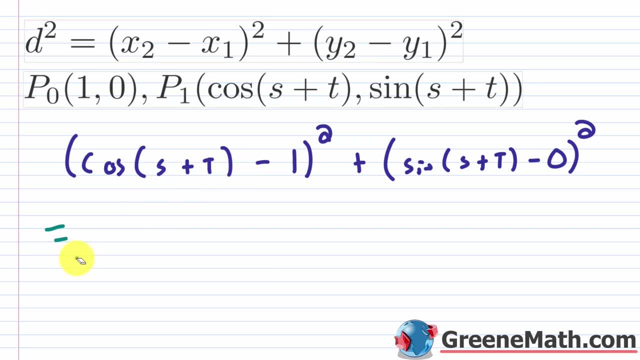 So I'm going to use my formula- Remember, if you have, let me just get rid of this for a second so I can write this out: So x minus y, quantity squared, this is x squared minus 2xy plus y squared. So we're just going to use that formula, pretty easy. So I'm just going to say: 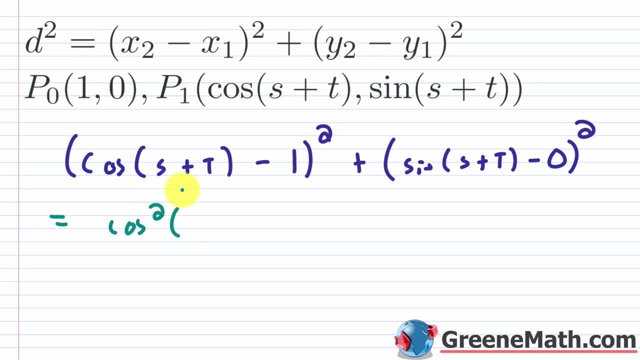 I have this first guy squared, so cosine squared, and then the angle would be s plus t there, And then minus two times this times this, Now, two times one is two, So it's just two times the cosine of this s plus t here, And then plus this last guy, one squared, which is just one. Now I'm 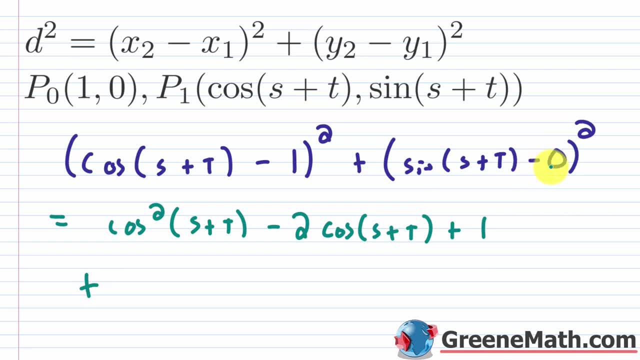 going to go plus. Now this one right here, because you have minus zero. you could really just get rid of this and just say you have sine of s plus t being squared, So I'm just going to write that as sine squared of this s plus t angle. So now we have 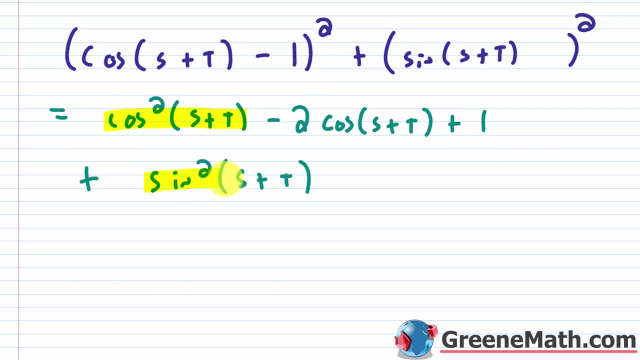 cosine squared of s plus t, And we have sine squared of s plus t. Remember, if the angle is the same, which we have s plus t and s plus t, well then cosine squared theta plus sine squared theta is equal to one. So this plus this would give me one. So really I can say that we would. 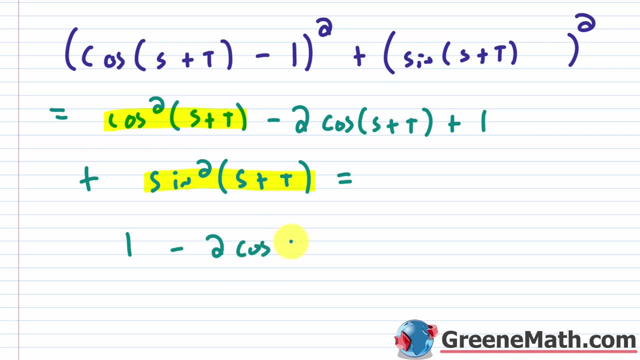 have one, and then we have minus two times the cosine of this s plus t, and then plus one. So this is going to give me a final result for this side: one plus one is two. So we'll say two minus two times the cosine of s plus t. Okay, let me grab this And I'm just going to paste this in: 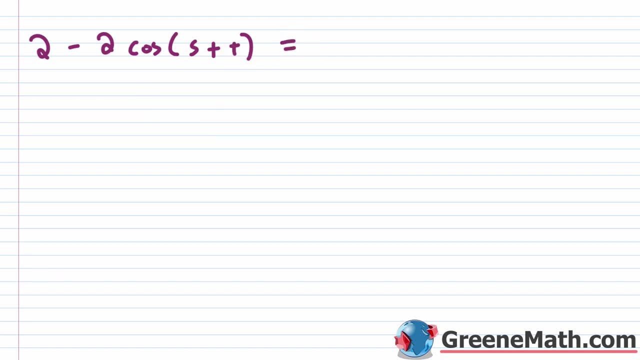 here. So this is one side. let me put equals, And now we're going to work on this side. So we have q sub zero and we have q sub one. So just plug in here. forget about the d squared equals. 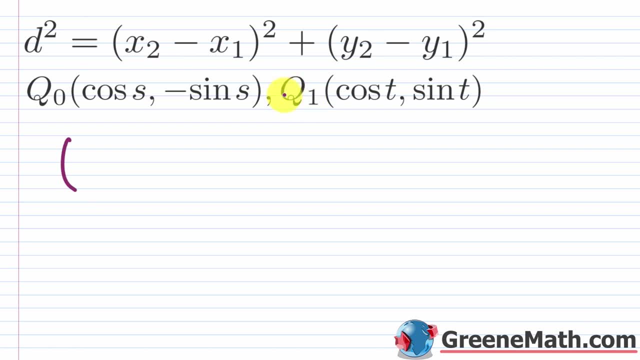 I'm just going to find the x sub two, which, again, I'm labeling this as the second point. So I want cosine of t. So then, minus, you want your x sub one. here that would be cosine of s. Let me close that down and square it. So then, plus, you have your y sub two. So here, 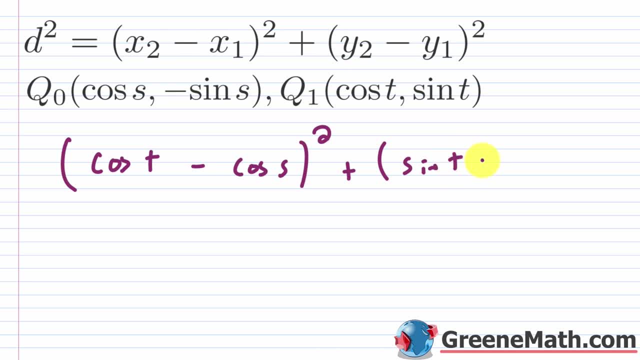 that's going to be the sine of t. So the sine of t. And then you have minus your y sub one. In this case that's going to be the negative of the sine of s. Now minus a negative is plus a positive, So you want to put a plus there and then the sine of s. So be very careful about that. 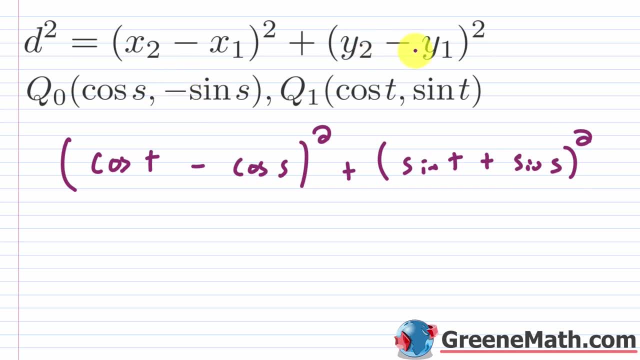 step there. A lot of people get confused. Remember this is right: here a minus And in the formula you have a minus. So minus a negative is plus a positive. That's why we have a plus there. Okay, so I'm just going to use my formula here, So we know the. 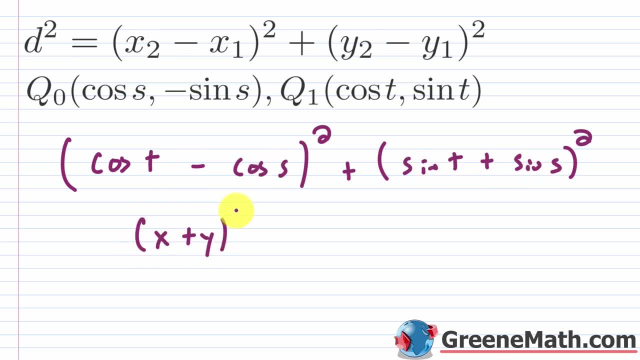 formula for this one And this one: if you have x plus y quantity squared, it's x squared plus two, x y plus y squared. Okay, if this changes to a minus, then only this changes to a minus. everything else is the same, Okay. so let's get rid of this And let's write equals here. 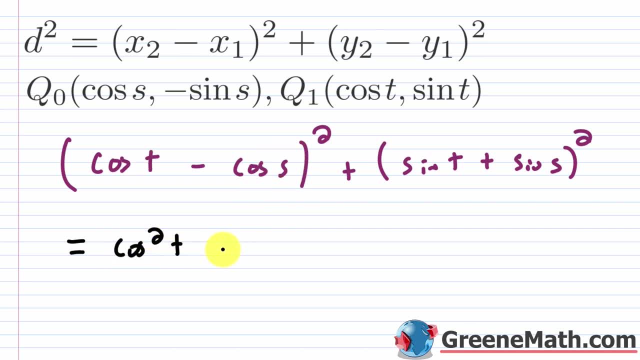 So this would be the first guy squared, which is cosine squared t, and then minus two times this guy times this guy. So the cosine of t times the cosine of s, And then plus the last guy squared, So this is cosine squared s. Okay, then plus, let's work on. 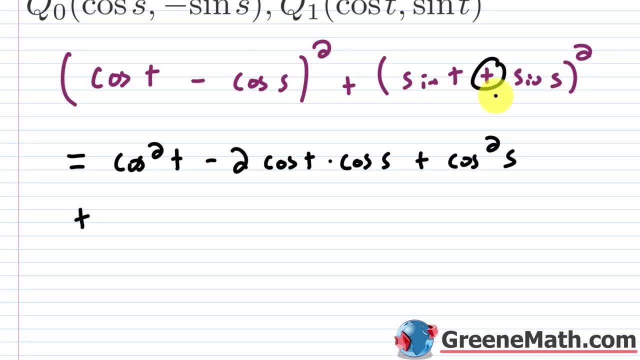 this guy. Now notice this is a plus guy here, right? So we have to think about a different formula. So the first guy squared, so sine squared t, then plus two times again the first guy times the second guy. So we'll put the sine of t times the sine of s and then plus the last guy squared. 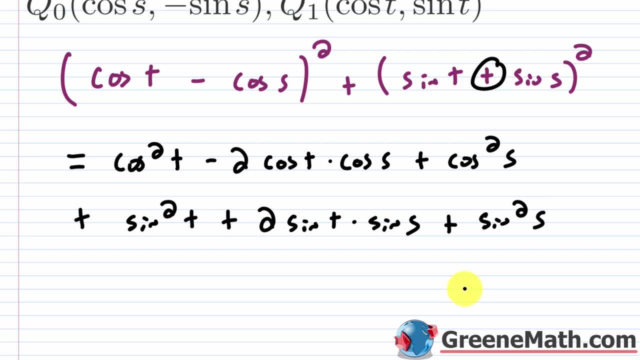 So this is sine squared s. Okay. so once again we have a situation where we can use that Pythagorean identity: sine squared theta plus cosine squared theta equals one. So cosine squared t and then sine squared t, So that's going to be one. And then let me highlight: 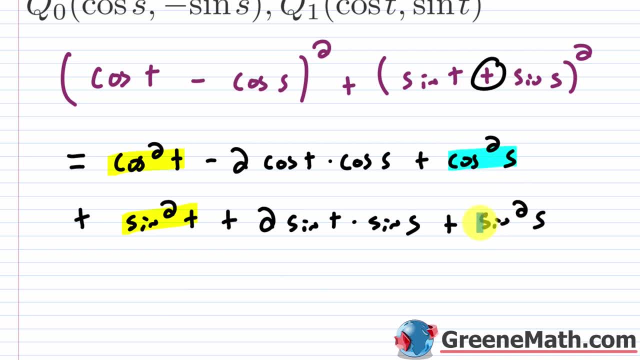 this in a different color. You also have cosine squared s and sine squared s. Okay, let's put equals. So we have cosine squared t plus sine squared t. as I just mentioned, that would be one. And then let's go ahead and say cosine squared s plus sine squared s. Let's just put plus one for. 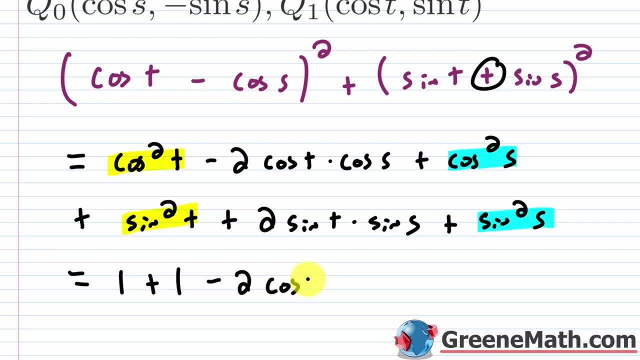 right now, And then we'll go minus two times the cosine of t Times the cosine of s, and then plus two times the sine of t times the sine of s. So we know that one plus one would be two. So instead of actually making a new line, 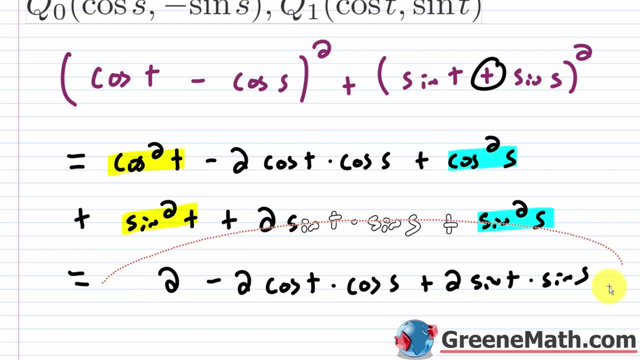 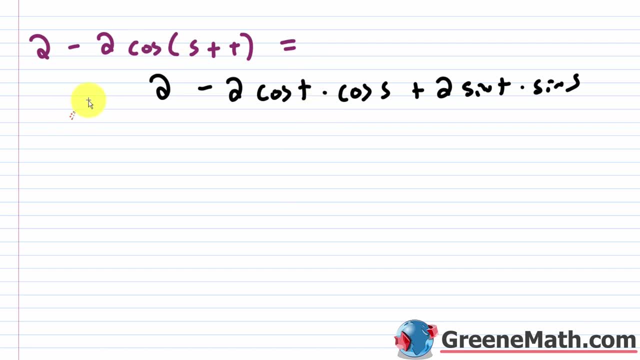 I'll just get rid of this and put a two here. That way we can speed this up. So I'm going to grab this and I'm going to paste this in here. It doesn't quite fit on one line, So we know that this is equal to this, What I would do. let me actually drag this a little bit further down. 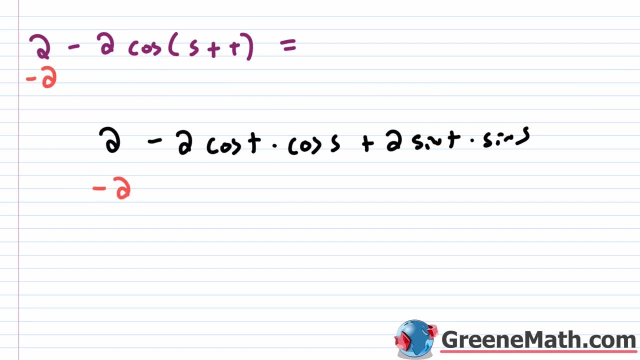 I am going to subtract two away from each side of this equation, So this right here is going to be two. So I'm going to subtract two away from each side of this equation, So this right here is going to cancel, and this is going to cancel. So let me see if I can write it in one line now. 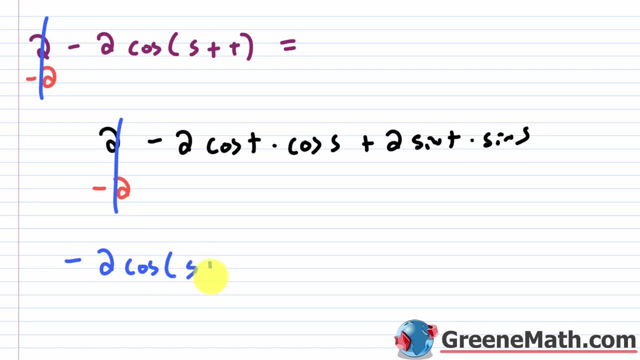 So negative two times the cosine of s plus t is equal to negative two. I'm going to flip the order here. for the purposes of the formula, You know that you can multiply in any order. So I'm going to say this is times the cosine of s, times the cosine of t. 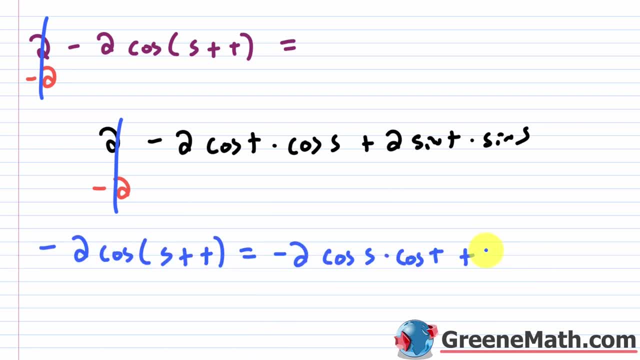 Then plus- let me slide this down and see if I can fit this- We're going to say two times your sine of s. Again, I'm flipping the order for the formula times- the sine of t. Let's come down here a little bit. 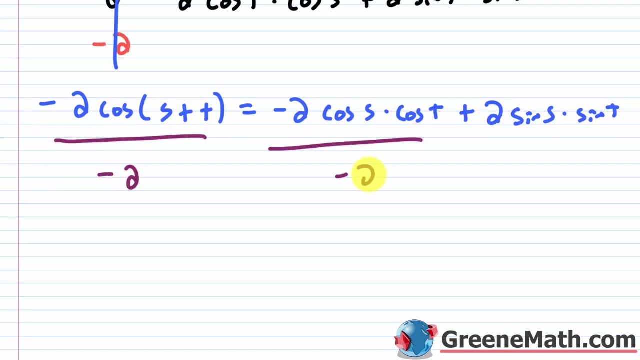 So what I'm going to do now is just divide everything by negative two, And that's going to get us where we need to go. So this is going to cancel And you'll have cosine of s plus t is equal to. this is going to cancel. 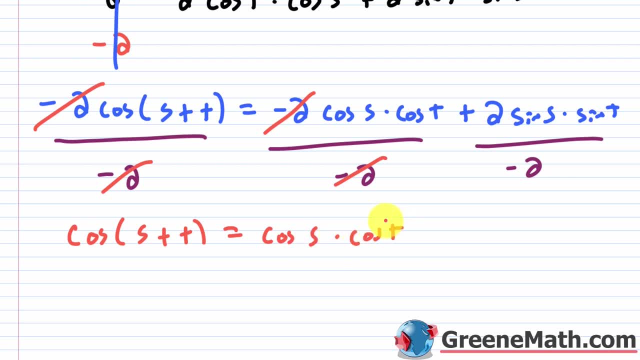 So you have the cosine of s times the cosine of t. Remember, it's the cosine of the first guy times the cosine of the second guy. Then positive over negative is going to be negative, right, You can think about this canceling, right? 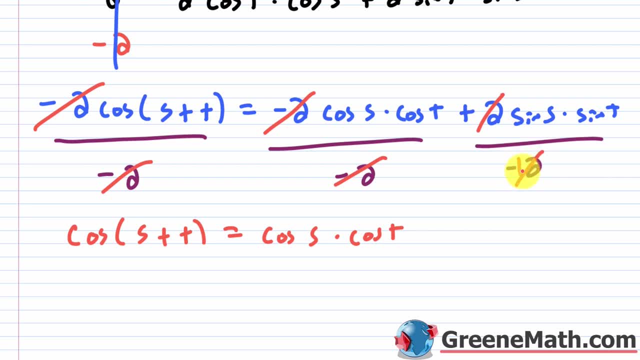 You think about this, canceling with this and giving you a negative one. So you basically divide by negative one or multiply by negative one, whatever you want to think about there, But essentially you have a minus here and then it's going to be the sine of s times, the sine of t. 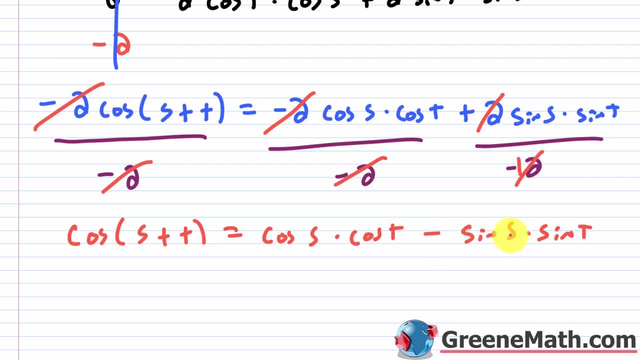 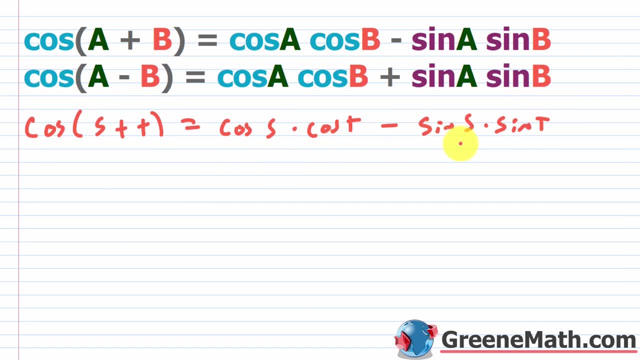 So again, your sine is different. You have a plus here and a minus here, And then it's the sine of the first guy times the sine of the second guy. If we grab this and we go back to our original formula, you see that it matches. 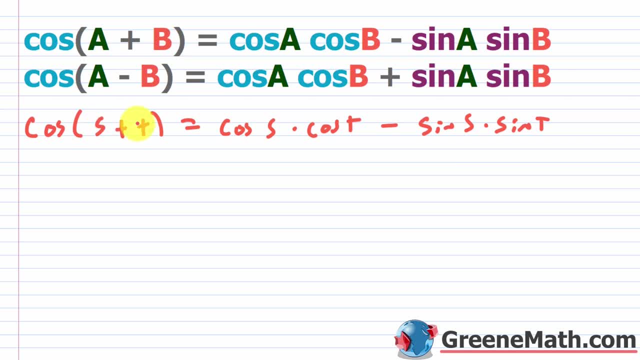 The only thing that's changed is the angle. Here we used a and b, Here we used s and t. So let me actually get rid of this. and I'm going to show you where the second one comes from. It's very easy if you understand the negative angle identities. 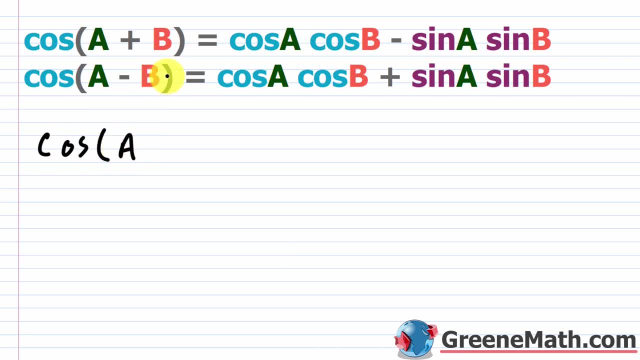 So let's say you said you had the cosine of a minus b, but you wrote it as a plus negative b, like this. So just following this formula here you would have the cosine of a, then times the cosine of this negative b. 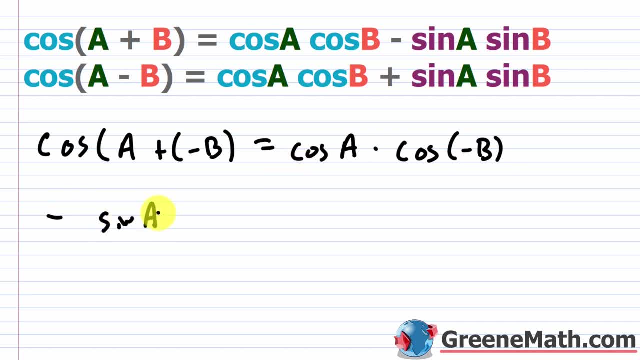 Then you would have, minus the sine of this, a times the sine of this, b, negative B With negative angle identities. again, the cosine of negative theta is the same thing as the cosine of theta And then the sine of negative theta is the same as the negative of the sine of. 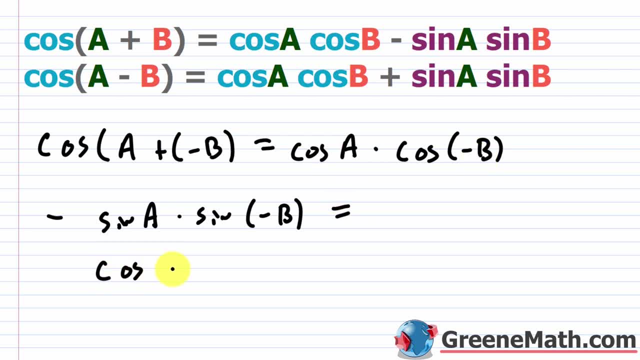 theta. So what I can do here is just say this is the cosine of A times the cosine of B, So that matches this part right here. Now this is going to come out right Because again this is the negative of the sine of B, So the negative times the negative would give me a positive, So I can. 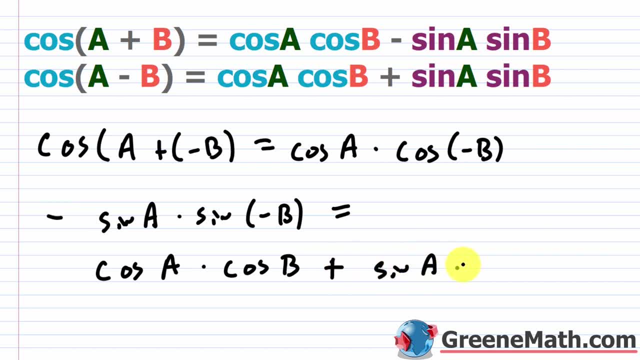 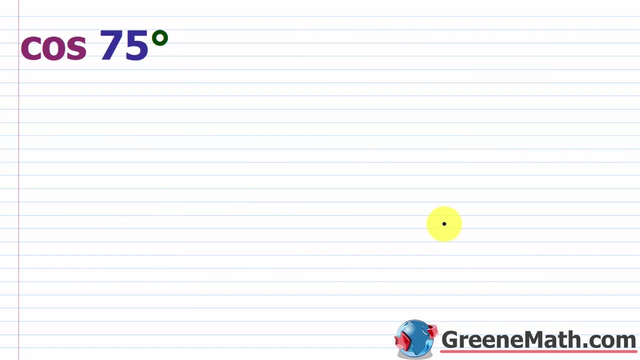 say: this is plus, now you would have the sine of A times the sine of B. So that's where this formula is coming from. Now let's look at a little example, And here we're given the cosine of 75 degrees. 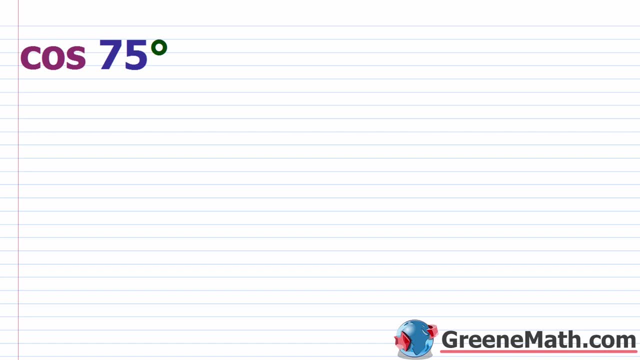 So this type of example, you're meant to give an exact value, okay. So the way you're going to do this is you're going to break 75 degrees up into two angles. that's going to be on the unit circle, okay, where you're going to know what this cosine value is going to be. So I can break this up one. 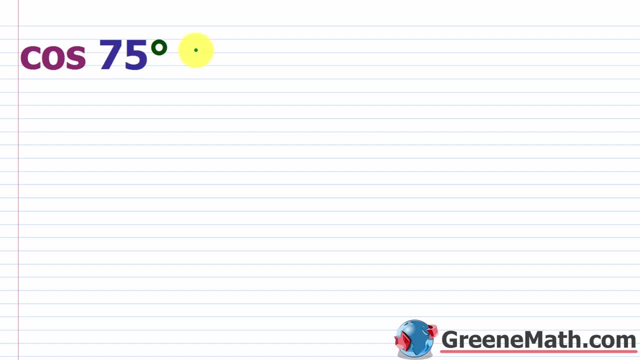 way to do it: 45 degrees and 30 degrees. So I'll just say this is equal to the cosine of, and I'm just going to go 45 degrees plus 30 degrees, okay, And then I'm just going to use my little formula. 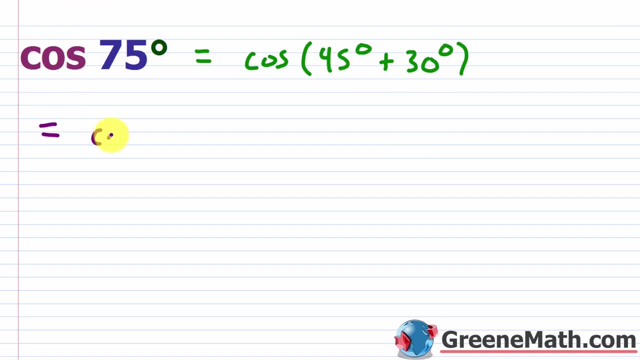 So we'll have what You want: the cosine of this guy. So the cosine of 45 degrees times the cosine of this guy, the 30 degrees, Remember, your sine is going to alternate. So because in this particular case we have a plus, we want a minus there. okay, So you want to change. 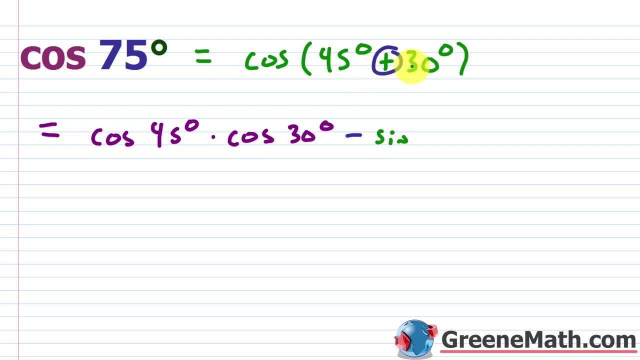 your sine. And then now I want to go with the sine of these two angles, So the sine of 45 degrees and then times the sine of 30 degrees. okay, So you're multiplying here. you're multiplying here, you're subtracting between the two. okay, So now what I want to do is just come through here. 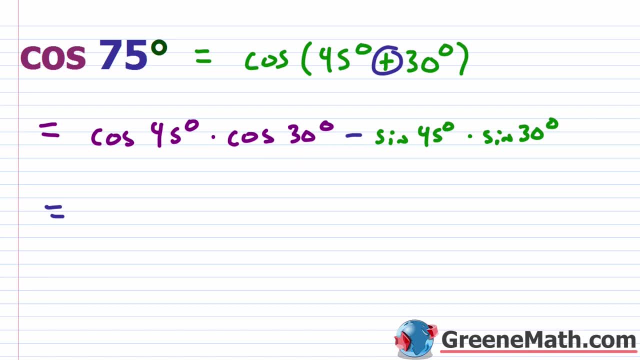 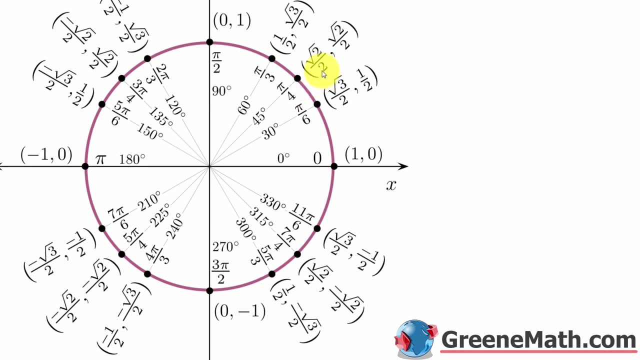 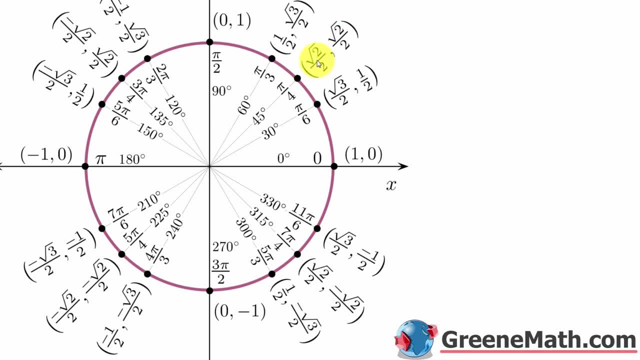 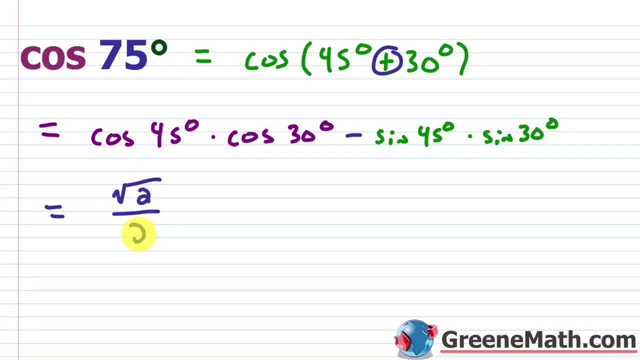 and then it's square root of two over two, for the sine, Remember, this is the x, that's the cosine, this is the y, that's your sine. So square root of two over two in each case. So this is square root of two over two and this is square root of two over two. okay, 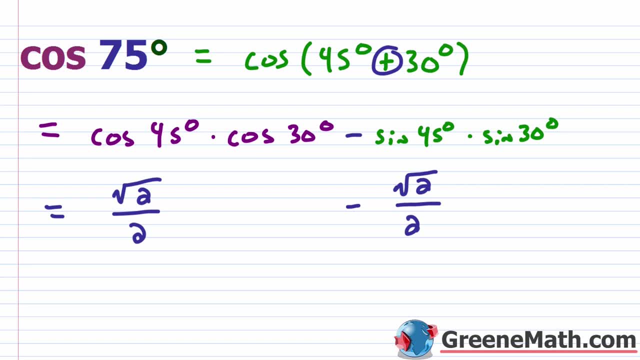 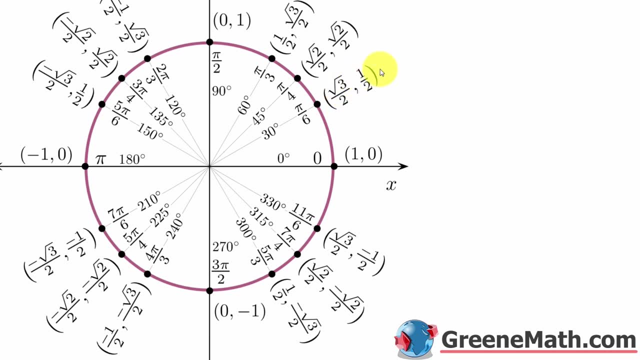 So what's going to be for 30 degrees? let's go back for 30 degrees, or pi over six in terms of radians. you've got square root of three over two for your x or your cosine, and then one half for your y or your sine. 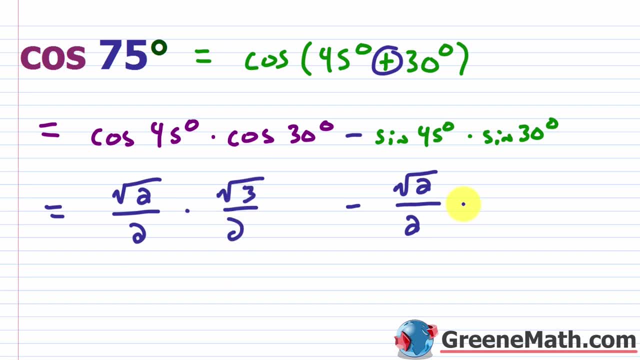 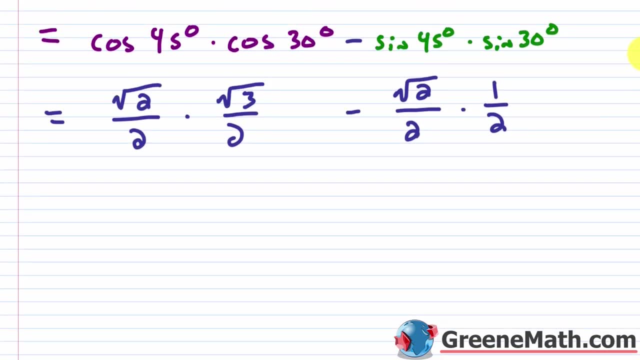 So this is going to be the square root of three over two, and this is going to be one half okay. So now all we have to do is just some basic arithmetic. So let's come down here a little bit, okay, And then let's switch the color here. 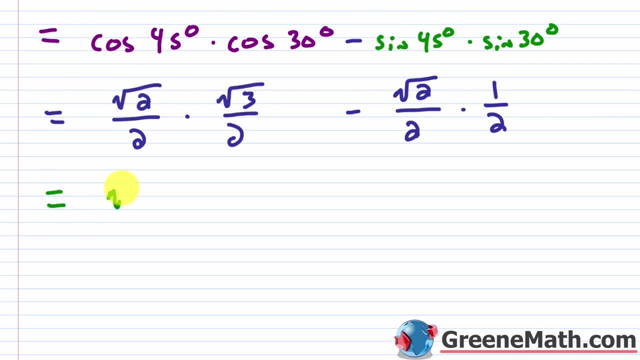 So this would be the square root of two times the square root of three. That would just be the square root of six over two times two, which is four. then, minus the square root of two times one, is just the square root of two. 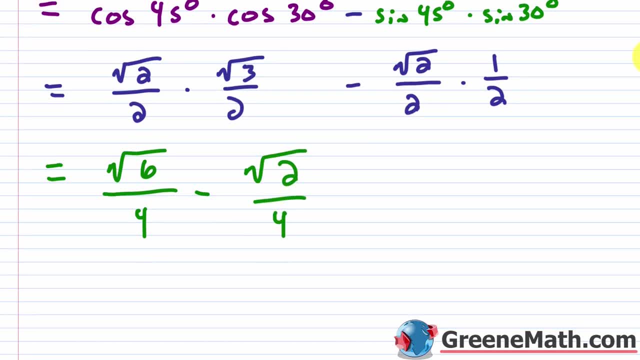 and then over two times two, which is four. Now, the only thing you can really do here is write this with a common denominator. So I'm just going to say that this is the square root of six minus the square root of two. 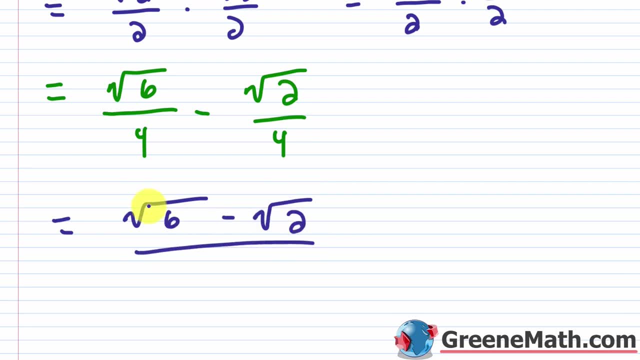 You can't combine there because the radicands are different. okay, You have the same index but different radicands, so you can't really combine those. So then this is over the common denominator of four, and this would be your exact value. 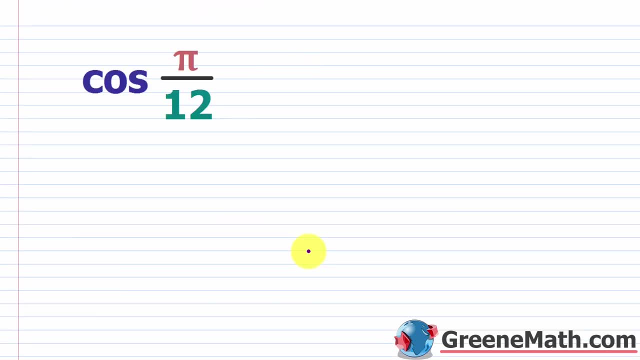 for the cosine of 75 degrees. All right, let's take a look at another example. So we're just trying to find the exact value again. So we have the cosine of pi over 12.. So obviously this is given in terms of radians. now 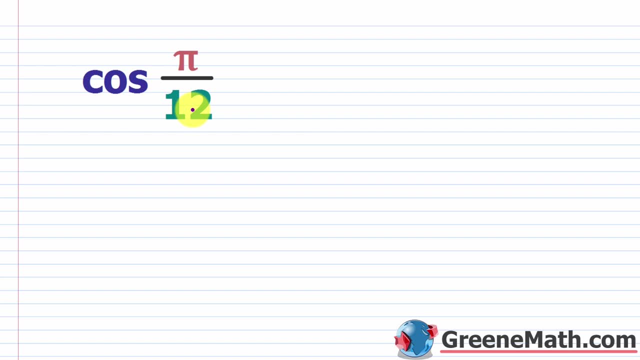 So what I'm going to do- and this is just a personal preference- I'm going to first convert this to degrees. It's a little bit easier for me to find two angles: to add or subtract, depending on what you want to do. 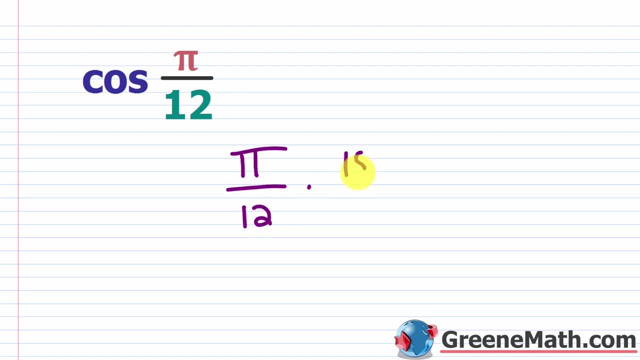 So I'm going to multiply pi over 12 in terms of radians times, 180 degrees over pi, And then basically I'm going to cancel this with this: 180 degrees divided by 12 would be 15 degrees, okay. So basically, if I had 15 degrees, 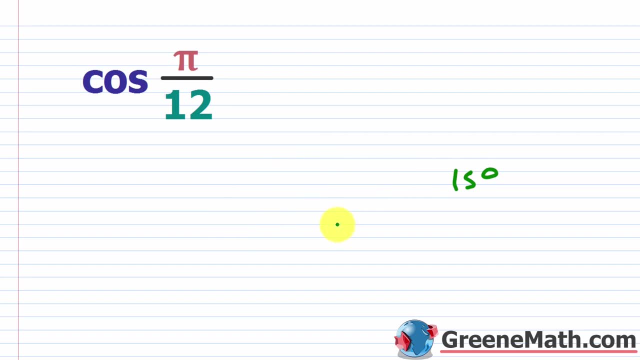 what I'd want to do is add and subtract. Let's say I did 45 degrees minus 30 degrees. That would give me 15 degrees. okay, So I could say this is the cosine of if this is in terms of radians. 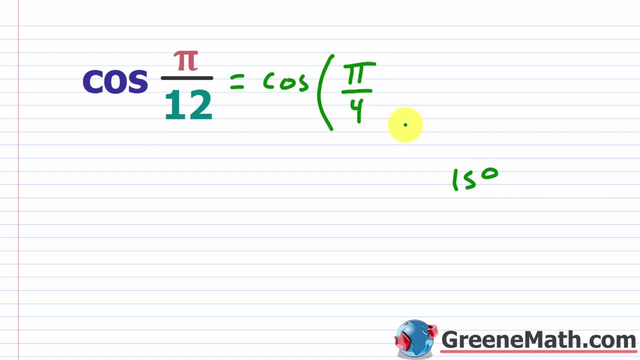 45 degrees is going to be pi over 4, okay, So pi over 4.. And then minus 30 degrees is going to be pi over 6, okay, in terms of radians. So I'm just going to use my formula from here. 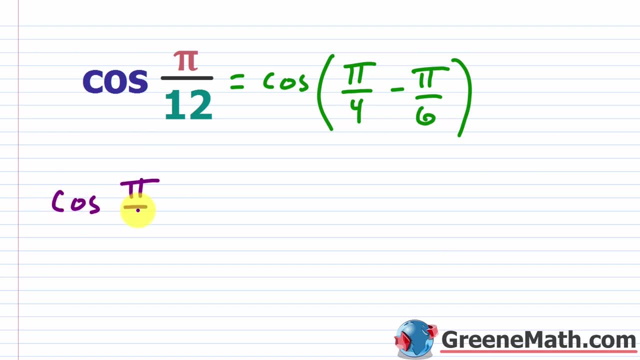 and just say that I have the cosine of pi over 4 times the cosine of pi over 6.. Because this is minus, I now want a plus. So I'm going to do the sine of pi over 4 and then times the sine of pi over 6, okay. 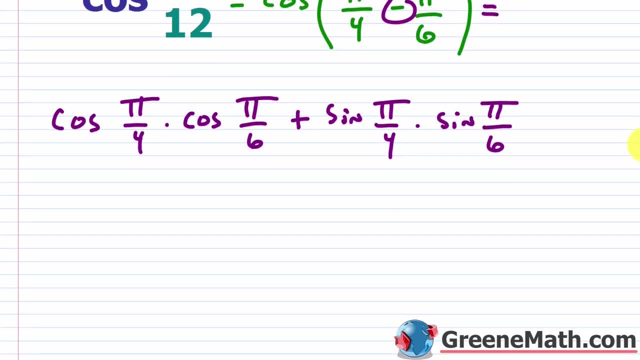 So let me put my equal sign there so we can keep going, And then I'll put equals over here. So if I think about pi over 4, or again 45 degrees, I know the cosine of 45 degrees and the sine of 45 degrees. 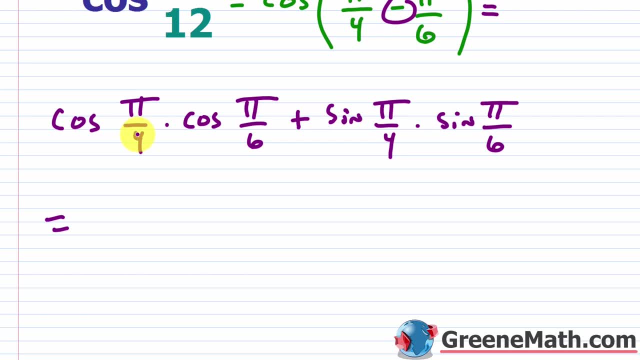 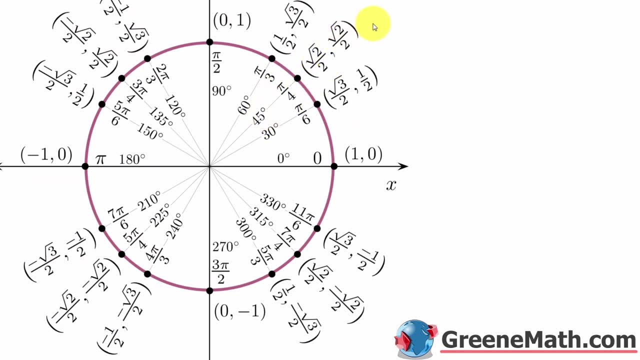 that's going to be the square root of 2 over 2 in each case. If I go back to my unit circle, you can see, for 45 degrees, or pi over 4, in terms of radians, we've got square root of 2 over 2 and square root of 2 over 2.. 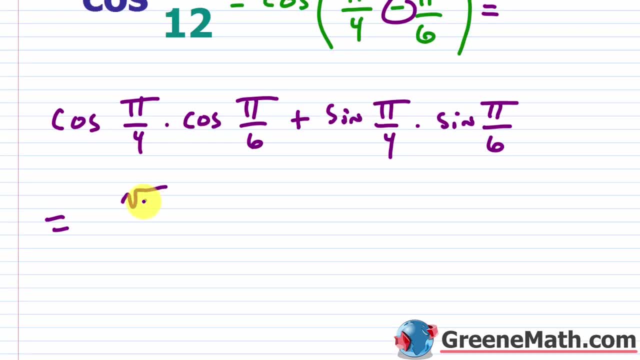 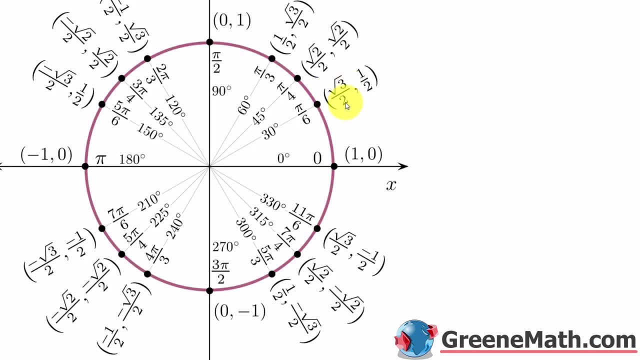 So let's go back and just replace this with the square root of 2 over 2 and the square root of 2 over 2.. Now for pi over 6 or 30 degrees we have again square root of 3 over 2 for the cosine and 1 half for the sine. 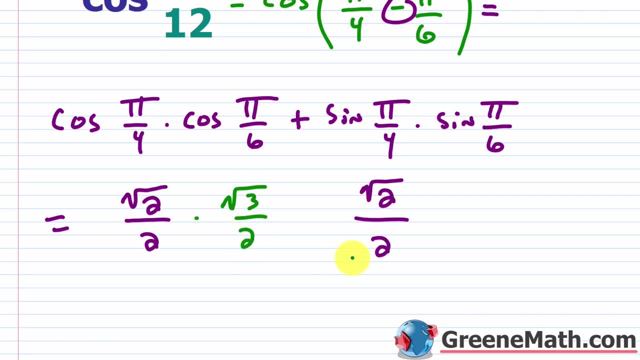 So this is going to be the square root of 3 over 2, and then we're going to have 1 half, and then I'm going to put a plus here between them. okay, So let's go ahead and scroll down a little bit. 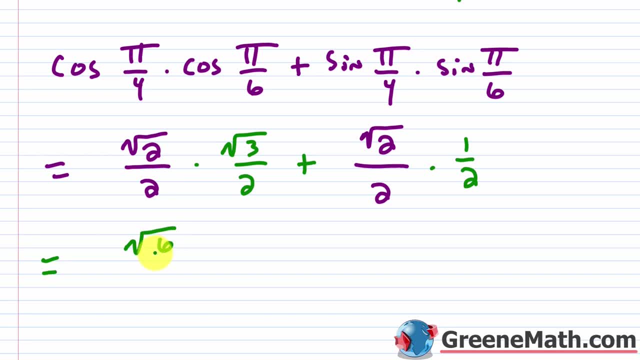 and do some arithmetic. So this would again be the square root of 6 over 4.. Now, plus now, I'm going to have the square root of 2 times 1, which is the square root of 2, over 2 times 2,, which is 4, okay. 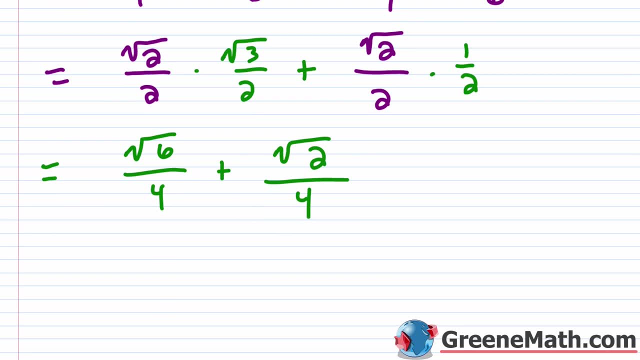 So again, pretty much all we're going to do here is: we're going to do this. So what I'm going to do here is just write this with a common denominator: I can't add the square root of 6 and the square root of 2.. 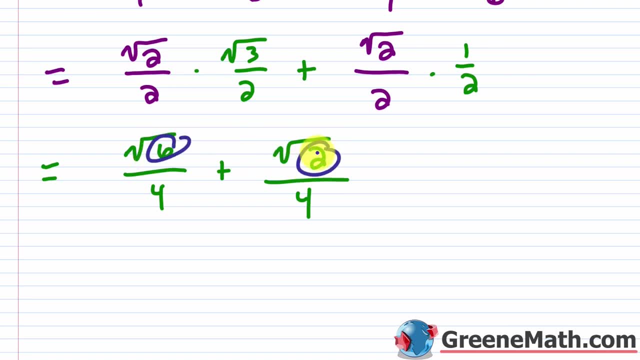 I can't combine those radicals there, because this and this is different, right? So you have different radicands, same index with different radicands. So I'm just going to write this as the square root of 6 plus the square root of 2 over the common denominator of 4.. 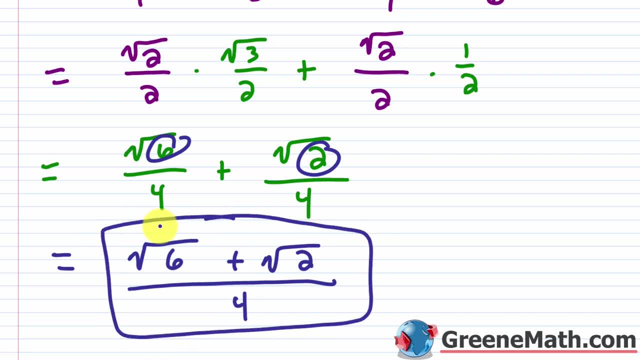 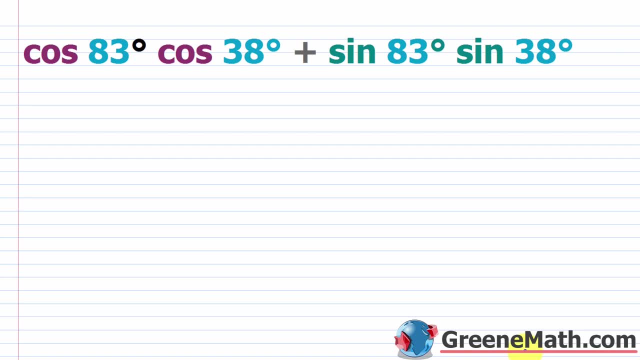 So this will be my cosine of pi over 12 radians. Okay, let's take a look at one more of these So you might see the problem that we just worked on those two problems rearranged. So now you see the cosine of 83 degrees times 2 times 3.. 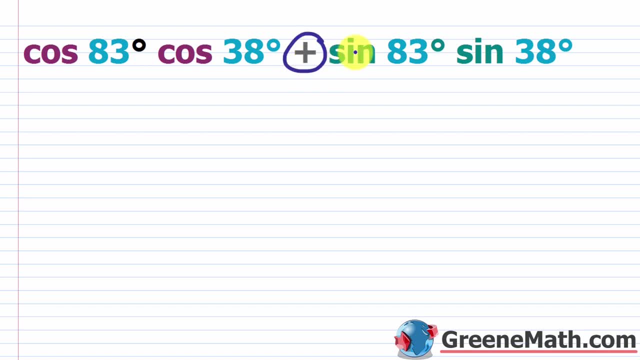 So this is the sine of 83 degrees times the cosine of 38 degrees, plus- this is the key here- the sine of 83 degrees times the sine of 38 degrees. So you see that you have the cosine of some angle times the cosine of some other angle. okay, 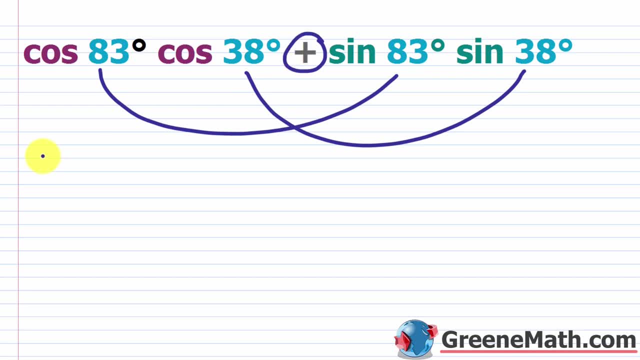 And then you have the sine of that first angle, so that angles here match, and then the sine of that other angle. okay, So the angles there match. You have a plus between them. You're meant to realize that you could write this. 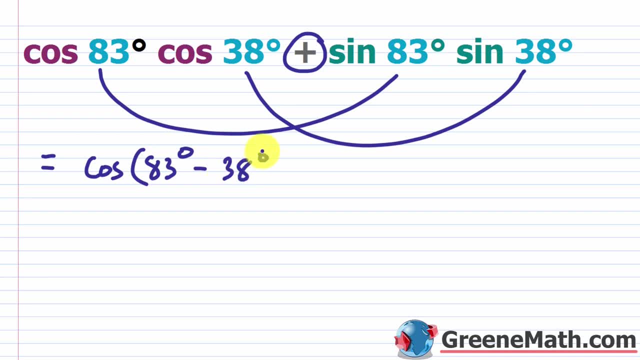 as the cosine of. again, this is a plus, so I want a minus degrees. Okay, so what is this going to be? If I do 83 degrees minus 38 degrees, I'm going to get 45 degrees. So this is the cosine of 45 degrees, And we already know, because we've done this in. 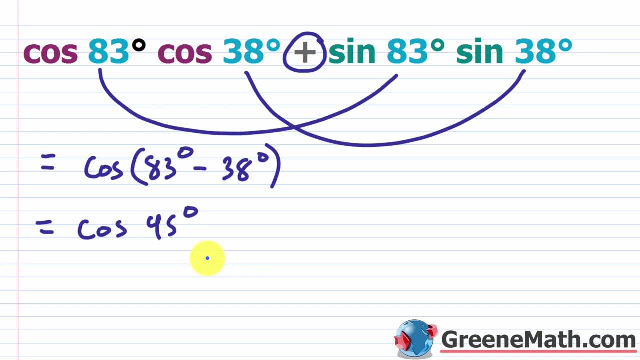 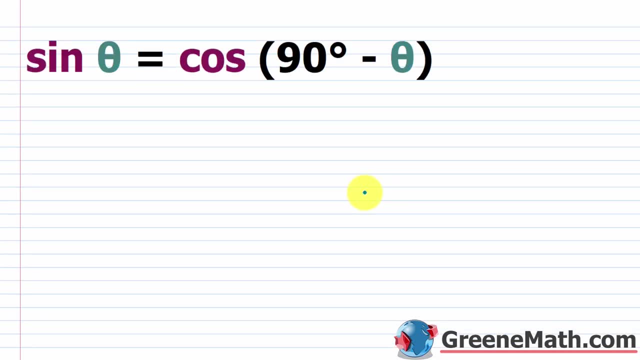 the last two examples that the cosine of 45 degrees is a square root of two over two. So this is exactly equal to the square root of two over two. Alright, so another thing that comes up in this section: we're going to revisit the co function identities. So before, when we looked at 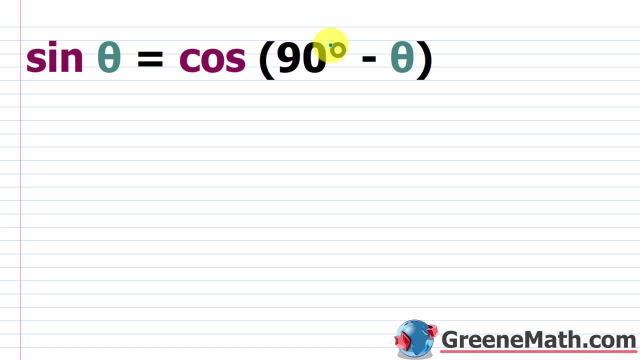 something like: the sine of theta is equal to the cosine of 90 degrees minus theta. we said that theta needed to be an acute angle, But now we're going to update that and say that theta can really be anything as long as the function is defined. So to prove this, what we're going to do is use: 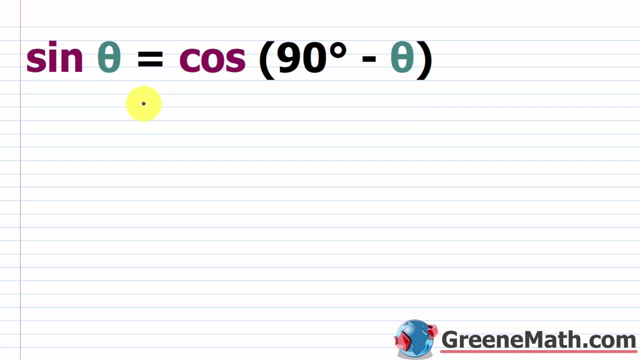 the cosine difference, identity. And over here let me just put equals here, And I'm going to say that this is the cosine of 90 degrees and then times the cosine of theta, And then again, if this is a minus, you want to use the cosine of theta, And then again, if this is a minus, you want to use. 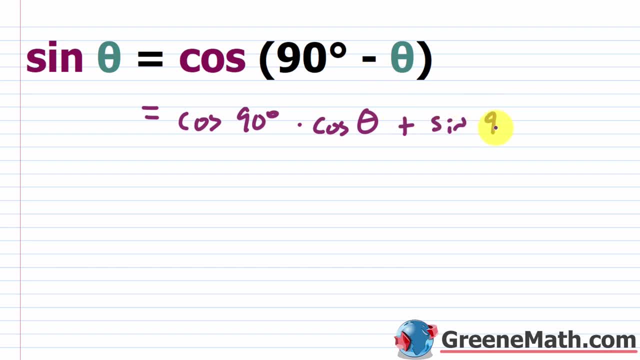 a plus here. this is the sine of 90 degrees and then times your sine of theta. Now we know that the cosine of 90 degrees is zero and zero times anything is zero. So you could write this out and say: this is zero times the cosine of theta And then, plus, we know the sine of 90 degrees is one. 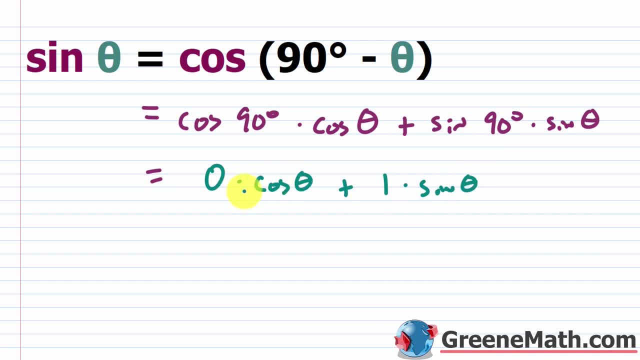 So this is one times the sine of theta, And so again, this is going to go away. So you're just left with one times the sine of theta, which is just the sine of theta. So you can see that this is going to work for any value of theta. Again, as long as the function is defined, you'll be good. 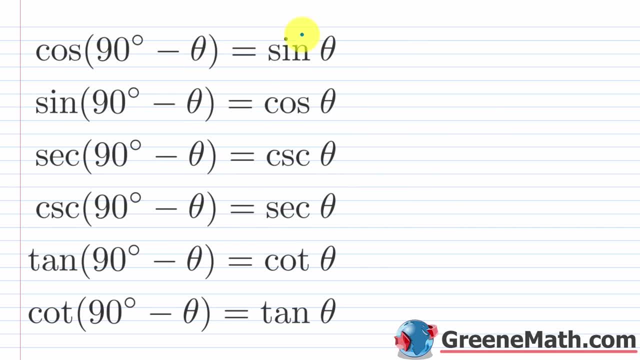 to go, So we can actually extend this to these other guys that we looked at earlier. So we have: the cosine of 90 degrees minus theta is equal to the sine of theta. the sine of 90 degrees minus theta is equal to the cosine of theta. Again, sine and cosine are co functions. Same thing for 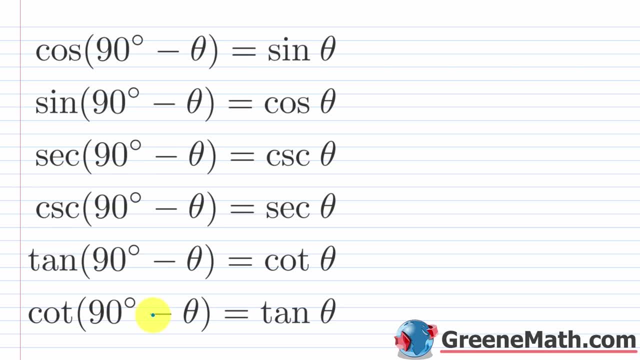 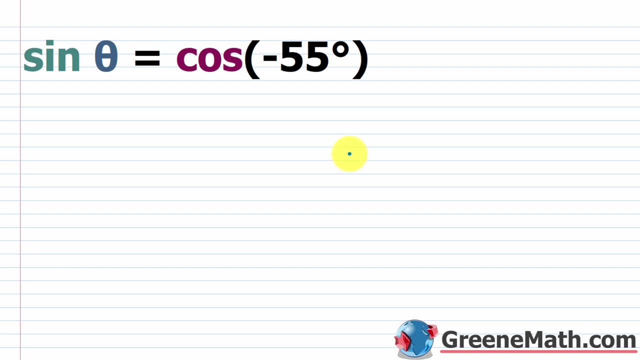 secant and cosecant And for tangent and co tangent. Now let's look at a little example. And we haven't gotten to solving trigonometric equations yet. We should know that the solution I'm going to give you here is one of many, many possible. 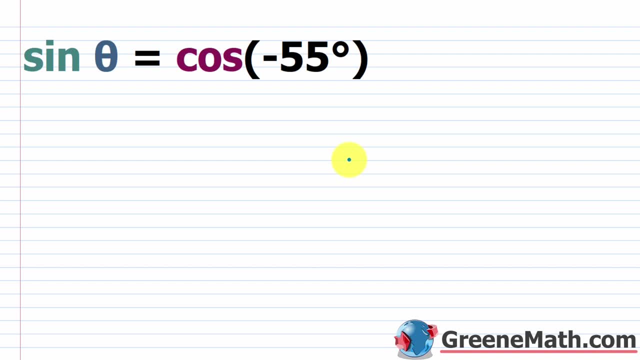 solutions, where you could say an infinite number of solutions, but I'm just going to give you one. So here we have. the sine of theta is equal to the cosine of negative 55 degrees. So what you'd want to do is write this left side in terms of cosine, so that you have cosine of some angle equals. 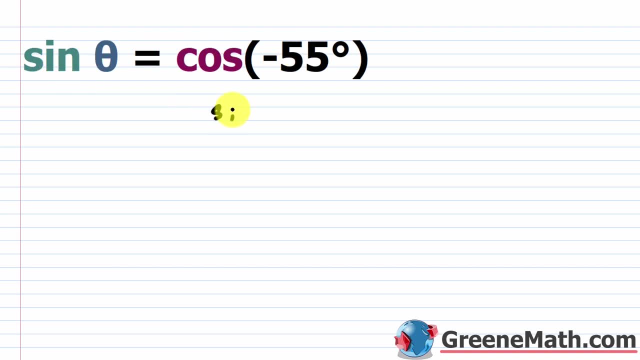 cosine of this angle here. So I know that the sine of theta is equal to the cosine of 90 degrees minus theta. So I'm just going to replace this guy right here with this guy right here, right, since they're equal. So I'm going to say that this is the cosine of 90 degrees minus theta. 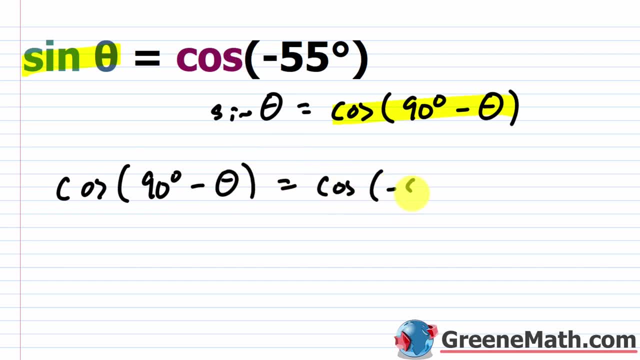 And this is equal to this guy right here, which is the cosine of negative 55 degrees. you get rid of this scratch work here and get rid of that Now. let me just slide this up here a little bit. And so what you would do here? you would set this guy equal to this guy, right. you set the angle measures equal, So we would say that 90 degrees of theta is equal to plata. Now, as I said a few minutes ago, you can put an equ 나오 tahj in there. So what I'm going to do here is I'm 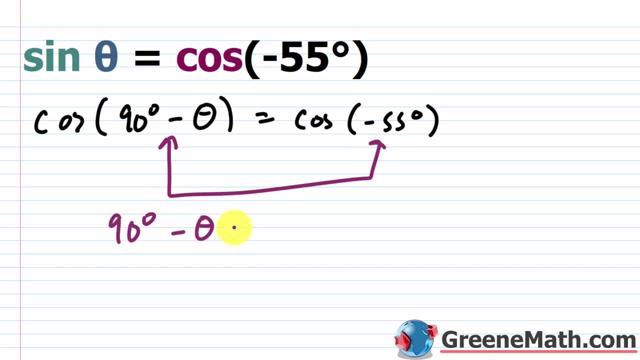 going to slip up this one row and it'll go right to this one row and that one row will get rid of the equal. So we would say that 90 degrees minus theta is equal to negative 55 degrees, And so let me subtract 90 degrees away from each side of the equation. this would cancel. slide down here just. 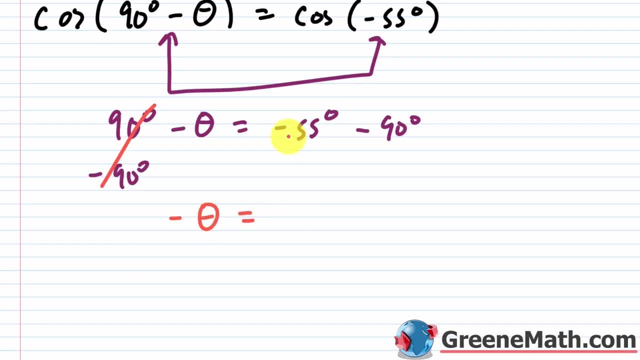 a little bit. we'll say the negative of theta is equal to negative 55 degrees minus 90 degrees, that's going to be negative 145 degrees. And then, to finish this up, I'll divide both sides of the equation by negative one. this would cancel. So you get: theta is equal to. this will be 145 degrees. 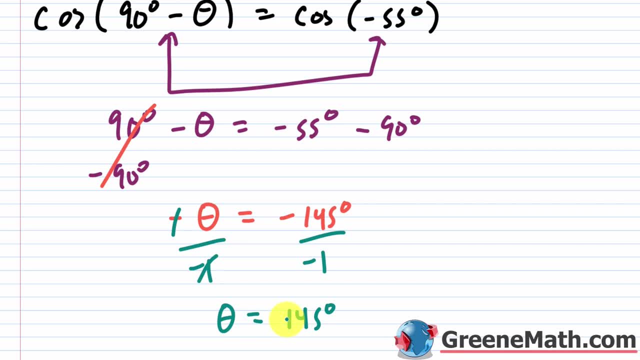 Now, again, this is not the only solution. Okay, again, when we get to solving trigonometric equations, we'll see that there's an infinite number of solutions. If you want, you can go back and plug this in And you'll see that the sine of 145 degrees is exactly equal to the cosine. 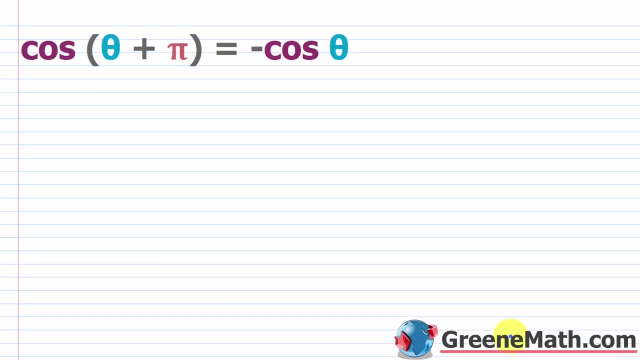 of negative 55 degrees. Okay, now let's look at two examples where we're going to verify some identities. These are a little bit easier than what we looked at in the last section, where we're strictly verifying identities. So let's start with. we have cosine of. 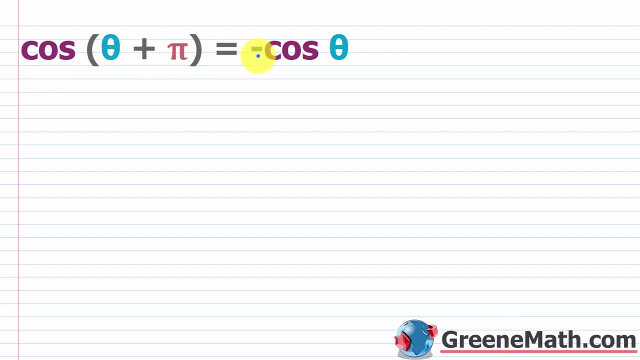 we have theta plus pi- okay, is equal to the negative of the cosine of theta. Okay, I'm going to flip this because the easier side is here on the right, So I'm going to write: the negative of the cosine of theta is equal to the cosine of: you have your theta, okay, plus your pi. Now what I'm? 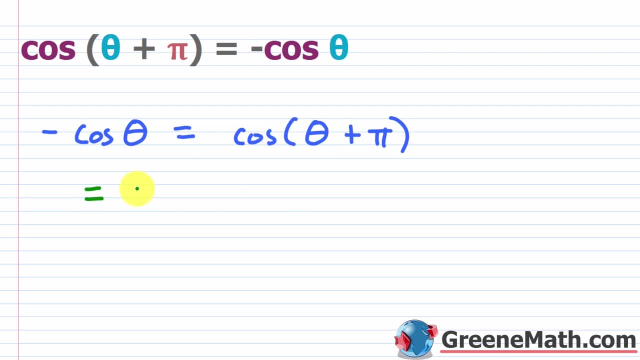 going to do is just put my equals over here. I'm just going to slide this over for formatting. okay, normally they put it in line, but I just want a lot of wrong, So I'm going to expand this out using the sum identity for cosine. So this is going to be negative of theta plus pi. okay. 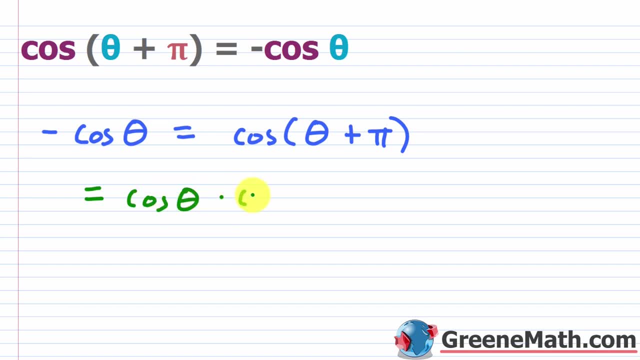 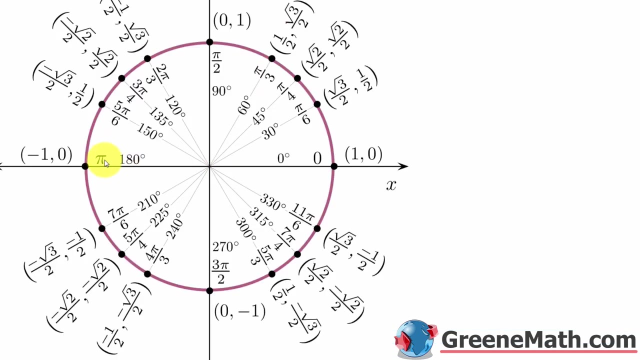 this would be the cosine of theta. okay, times your cosine of pi. And then remember, this is plus, you want to minus. so I'm going to go: the sine of theta times the sine of pi. Okay, now realize when you work with the cosine of pi or the sine of pi. let's go back to the unit circle. when we look at, 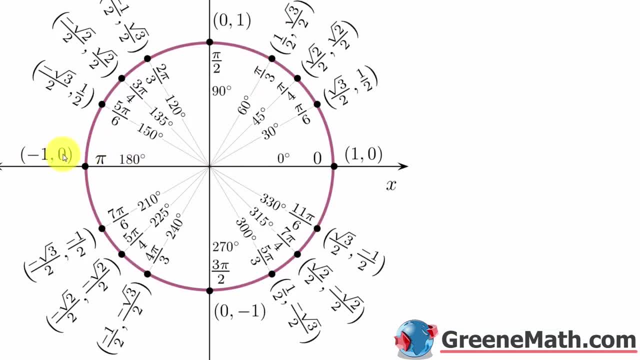 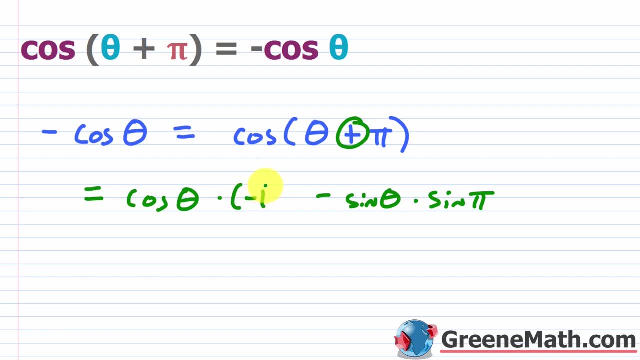 pi over here. the cosine is negative one, okay, and the sine is zero. So let's minimize this. So the cosine of pi is negative one, So let's put times negative one like this: And the sine of pi is zero, okay. so we know, if you multiply anything by zero, it's going to be zero, right. 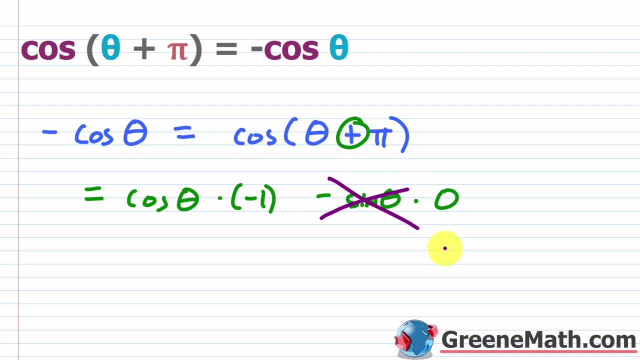 So basically, you can get rid of this part right here. right, you'd have minus zero, which is just gone. So basically I can say this is equal to the negative of the cosine of theta, And so that matches exactly what we have here, right? negative cosine of theta, negative cosine of theta. So 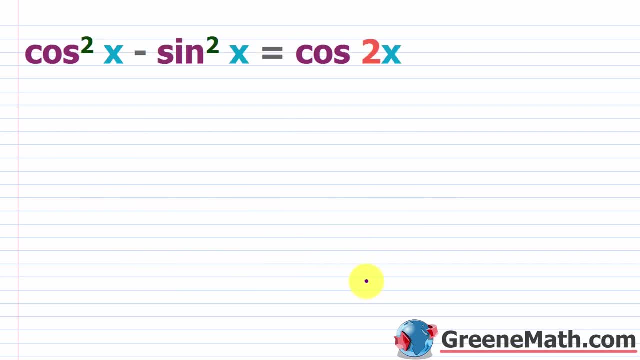 we're done. Okay, let's look at another example of verifying an identity. This one's just as easy. You have the cosine squared x minus the sine squared x equals cosine of two x. Now, if it's not immediately obvious what you need to do, remember if you have two x. 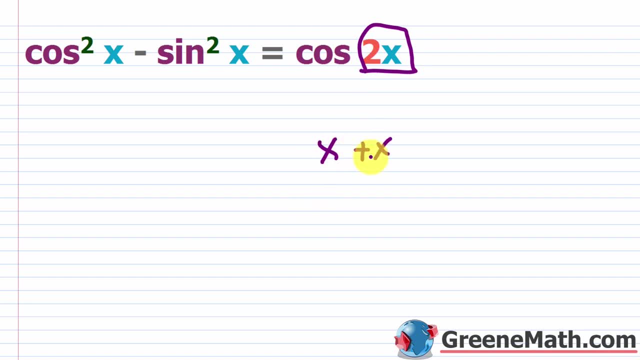 this is the same as x plus x, Okay. so if you're in this section, you're looking to think about the sum and difference identities for cosine, So think about things you can add or subtract. So two x is x plus x, Okay. so what I'm going to do here, let's just go ahead and put equals here. 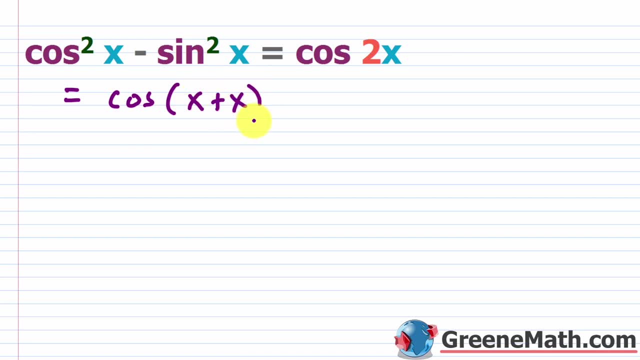 I'm going to write cosine of x plus x, like this, okay, And then I'm going to use my sum identity for cosine. So I'm going to say this is the cosine of x times the cosine of x. again, then minus, remember, this is plus, this is minus the sine of x times the sine. 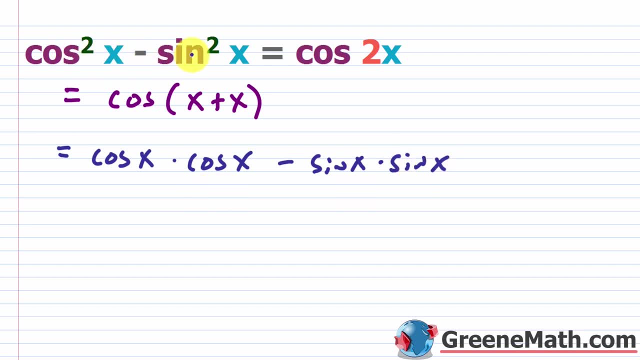 of x again. okay. So once you write it like this, it's clear that this is going to match right, Because cosine of x times cosine of x, I can say this is the cosine squared of x, And then, minus, I can say: sine of x times sine of x is sine squared of x. And now I can see that this side 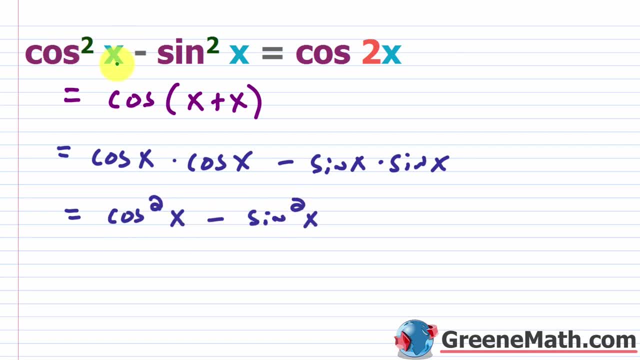 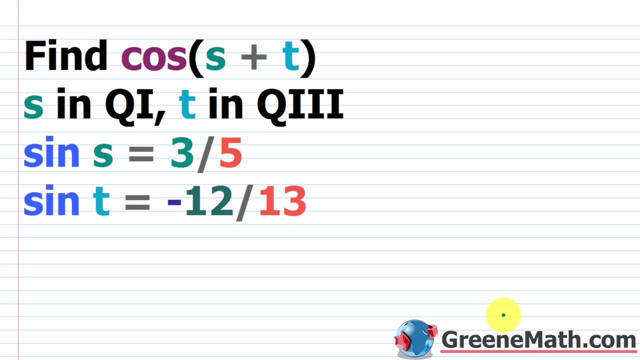 matches this side right: cosine squared x minus sine squared x. cosine squared x minus sine squared x. So I can put my checkmark there and I'm done. Okay, let's look at one more problem type that you're going to see. So we're asked to find the. 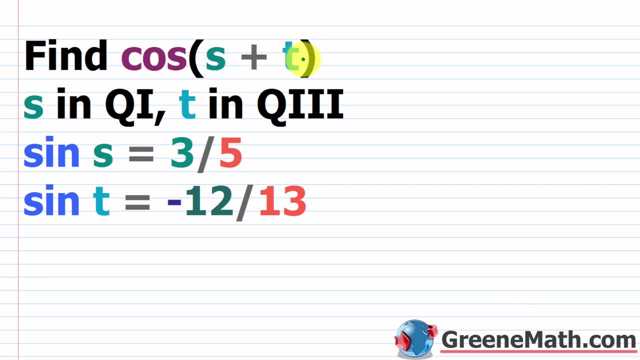 cosine of s plus t. you might also get the cosine of s minus t. the procedure, the way you do this type of problem, is the same. okay, So you have s in quadrant one and t in quadrant three. So they're giving you information about sine. So the sine of s is three fifths. the sine of t is negative, 12. 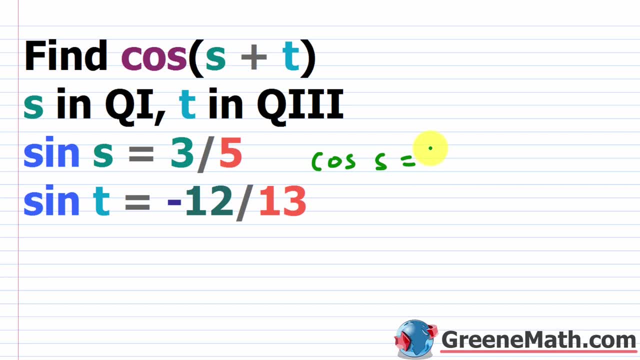 thirteenths. So the first thing we want to do is find the cosine of s, so that equals what, and the cosine of t, so that equals what. So one way you could do this is you could use your Pythagorean identity. Remember cosine in this case, let's say squared of s. 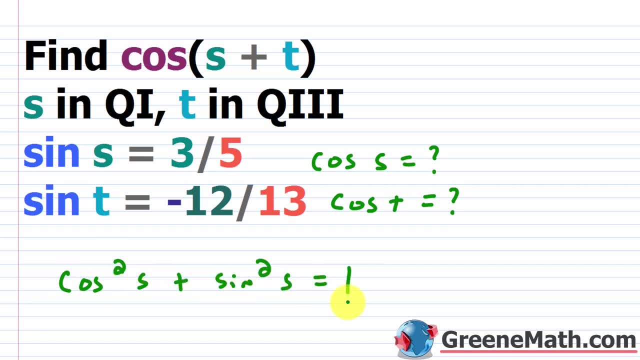 plus sine. squared of s is equal to one. okay, So if I plug in for sine of s right here, I can figure out what cosine of s is. okay, So let's scroll down, we'll come back up. So this is going to be three fifths. So remember, this guy is squared, So I'm going to plug in a three. 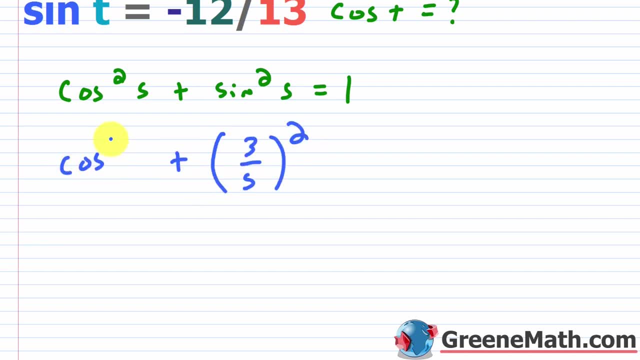 fifths here and I'm going to square that. So plus you have your cosine, squared of s and this equals one, okay, So three fifths squared, it's going to be nine, twenty-fifths. So this is nine twenty-fifths, So plus you have your cosine. 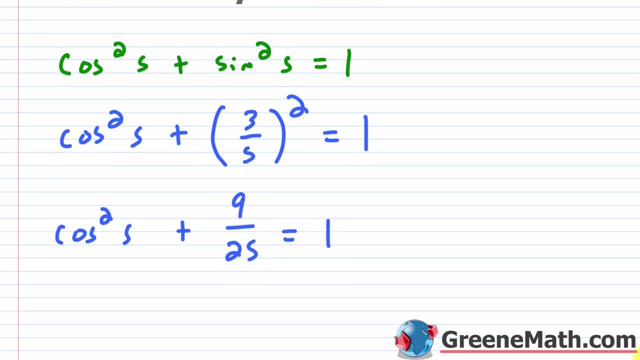 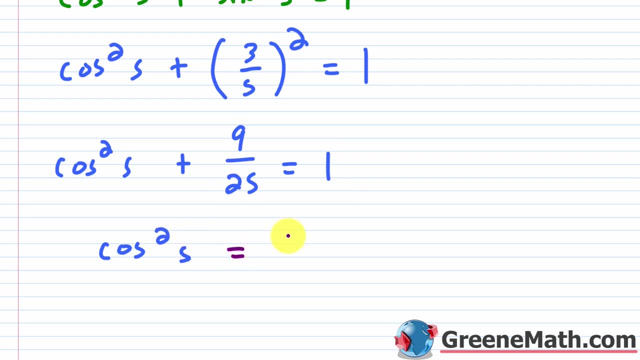 squared s here and this equals one. okay, So I'm going to subtract that away from each side. So I'm going to have the cosine: squared of s is going to be equal to. I'll go ahead and write one as 25 over 25.. So I have a common denominator and I'm going to subtract away nine over 25,. 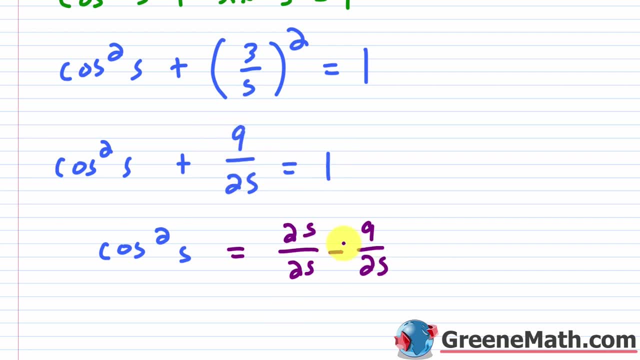 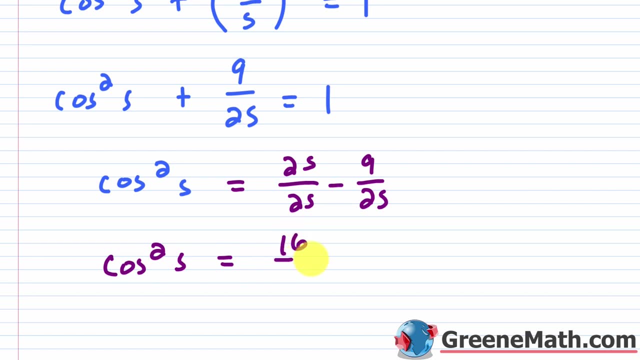 right, I'm just subtracting this away from each side. So 25 minus nine is going to give me 16, and so I'll say I have cosine. squared s is equal to: again, this is 16 over 25.. If I want cosine by, 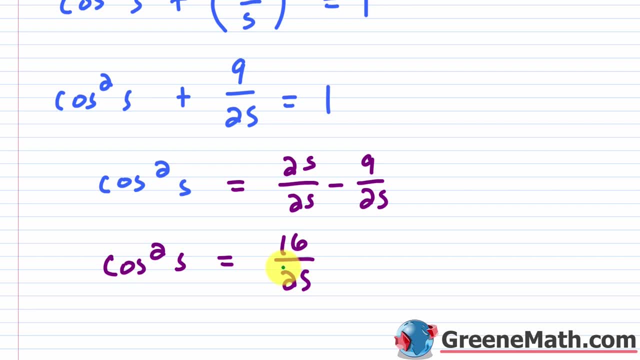 itself. I'm going to take the square root of this side. Again, you do plus or minus, but because we're in quadrant one for s, it tells us that I just want the principal square root of this guy. so I can erase this and just say I have, cosine of s is equal to this, And so cosine of s will be. 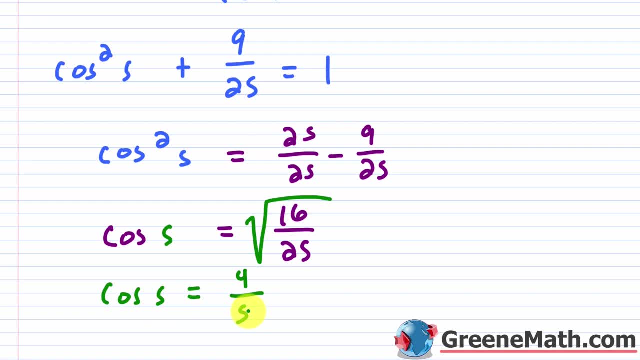 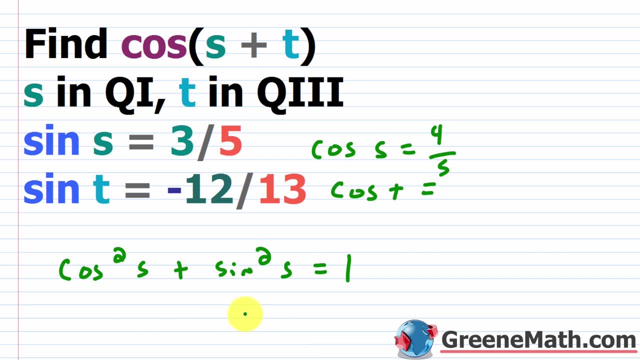 the square root of 16 is four. the square root of 25 is five. So you get four fifths there. So this guy is going to be four. okay, What about the cosine of t? Well, let's figure that out using the same process. Let's. 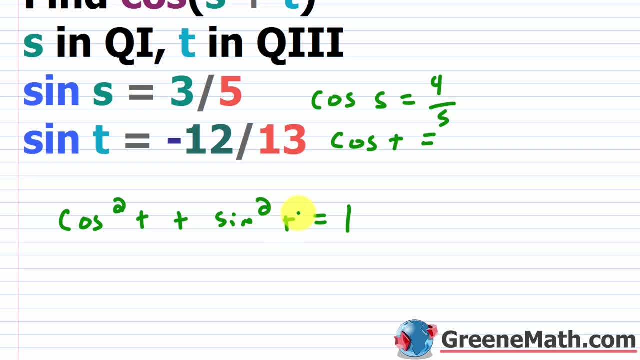 just change up this formula and I'm going to put t here and t here. It's the same thing. I'm just going to plug in for this. so negative 12 thirteenths, but t is in quadrant three now. 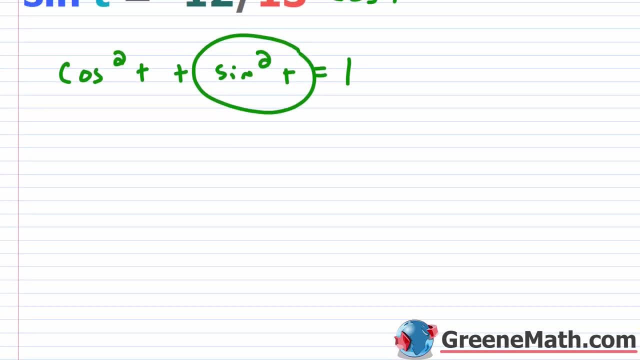 so keep that in mind. So let's come down here and let's plug in, So we're going to have the cosine squared of t, then plus, and I hate using t because it gets confusing with this plus symbol. So let me use the plus symbol in, like black or something, so it's clear that this is a plus. 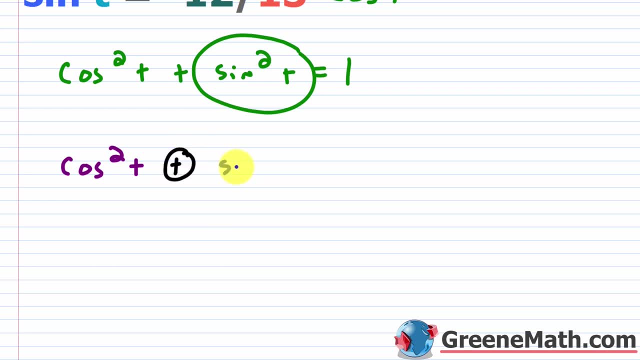 Even circle it. That's a plus, okay, So then we have the sine squared: t is equal to one. I'm plugging in a negative 12 thirteenths there, so negative 12 thirteenths and this guy's being. 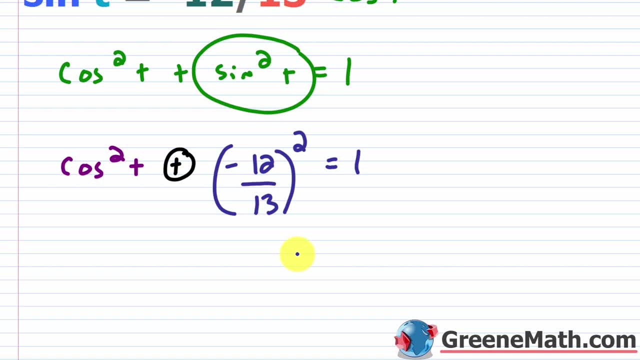 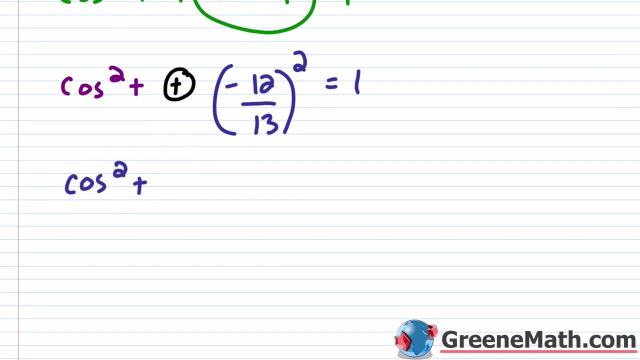 squared. So if I square a negative, I get a positive. If I square 12,, I get 144.. If I square 13,, I get 169.. So I'm going to say this is cosine squared t, and then- let me be careful, I'm going 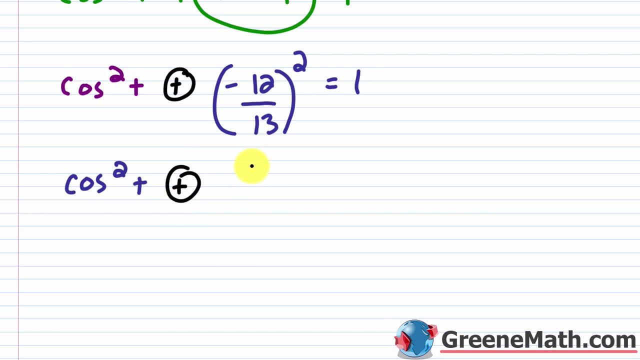 to put the plus sign here. Okay, again, that's a plus, and then this is going to be 144 over 169. And then this is equal to one. Okay, I'm going to subtract this away from each side And before I. 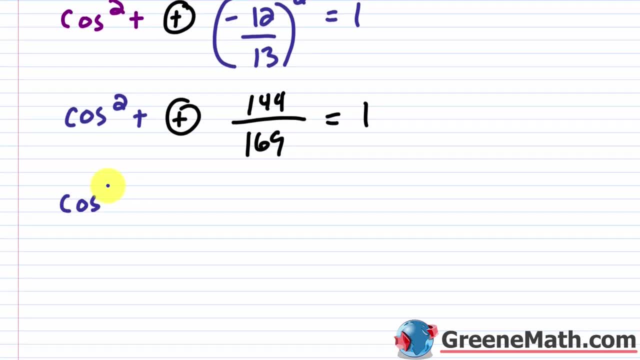 do that. let me just get a common denominator going. So let's go, cosine squared t. Okay, this is going to go over here. So I'm going to put equals and I'm going to do 169 over 169.. So 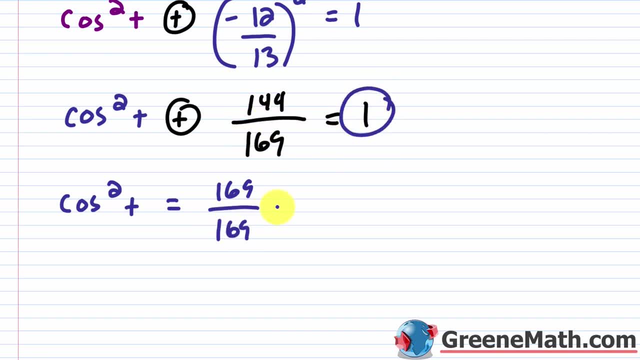 that's one. It just wrote it with a with a common denominator with this guy. then minus again. I'm subtracting this away from each side: 144 over 169.. Okay so if I do 169 minus 144, I get 25.. 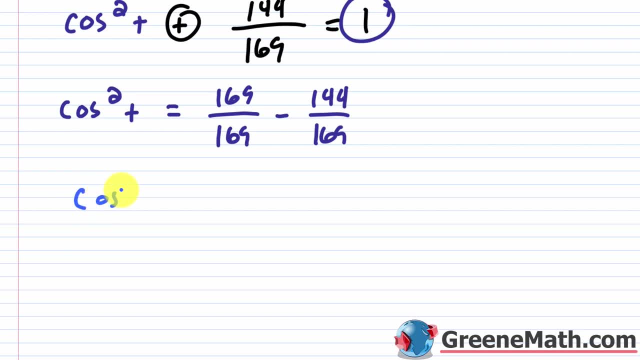 So let's scroll down just a little bit And we'll say that cosine squared of t is equal to: again, this is going to be 25 over 169.. Now, because we're going to be in quadrant three in terms of this t guy here, cosine is going to be negative. Okay, so I want the negative square root when I 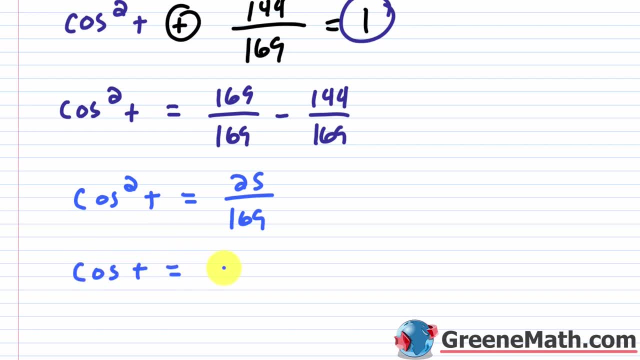 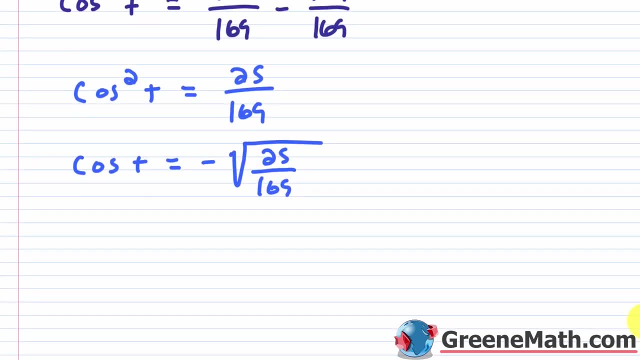 do this side. So I'm going to say cosine of t is equal to the negative of the square root of 25 over 169.. So let's go ahead and simplify that. So we'll say the cosine squared t is equal to, t is equal to. we'll have: the square root of 25 is five. the square root of 169 is 13.. So the 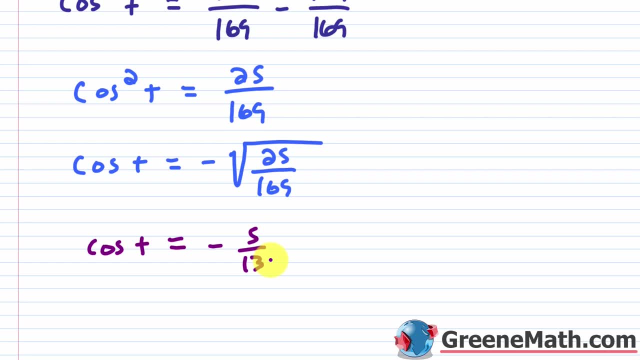 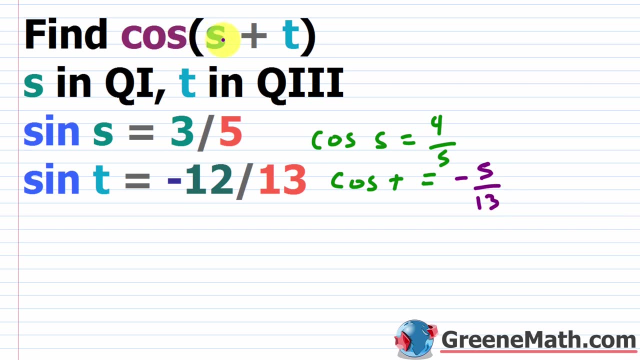 negative of five over 13.. Okay, so that's gonna be my cosine of t. Okay, so let's put negative five over 13, like this. So, now that you have all the information, you can find cosine of s plus t. So 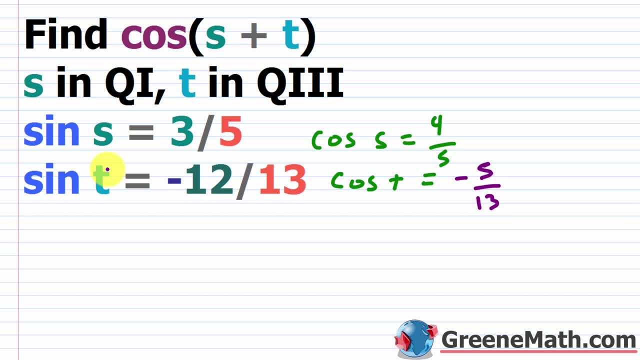 sometimes they give you sine of one of them and cosine of the other. Sometimes they give you sine of one and then sine of the other, Just depending on the situation you're given. you want to just plug into the identities that you know about. come up with some of the things that you know about. 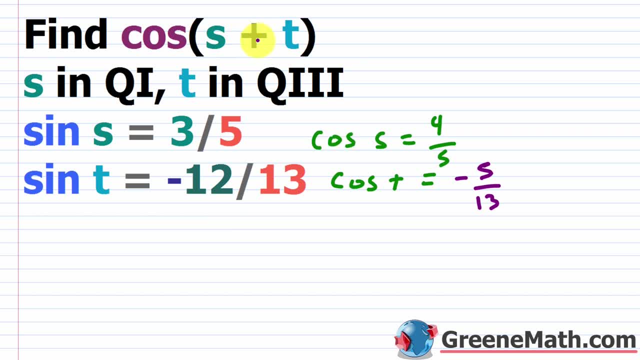 sine cosine of each of the angles And then you can go through and use your sum or difference identities, depending on the problem. Here we're going to use the sum identity for cosine And I'm just going to say that we have cosine of our s plus t is equal to again, if I take my cosine of s. 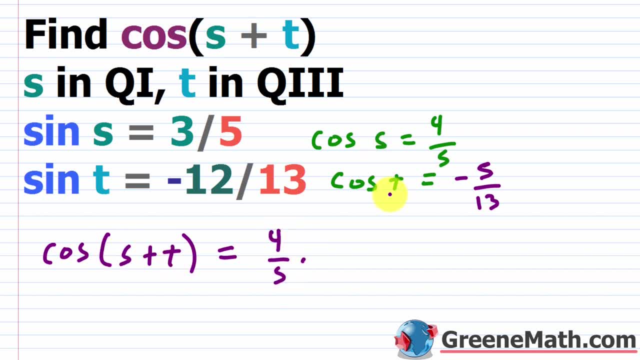 I know what that is. that's four fifths, then times my cosine of t. that's negative five over 13.. This is a plus here, Okay, so I want to make sure this is a minus. you're gonna be really careful. 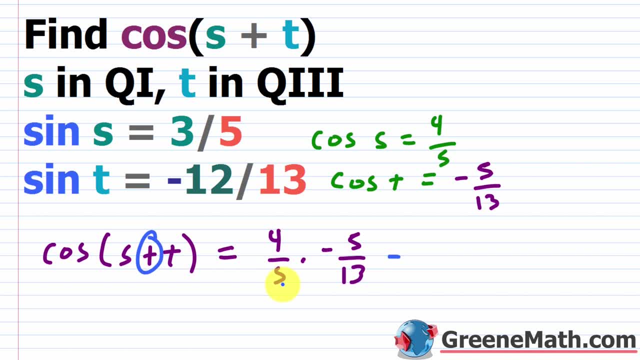 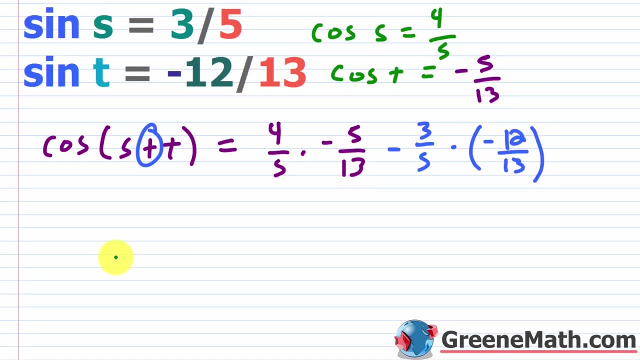 with the signs here, because sometimes you'll make a mistake with that. So now I want the sine of s, which is three fifths, Okay. And then I want times the sine of t, which is going to be negative 12 thirteenths Okay. So let's come down here a minute and just process this arithmetic. So I'm 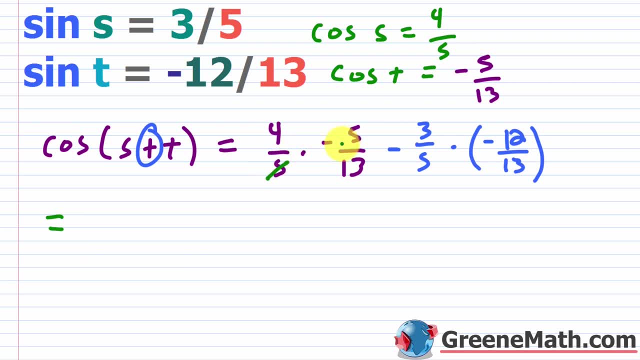 going to say this is equal to: if I multiply here, you see that this five would cancel with this five. So basically I have a negative one there. Okay, So this is basically negative four over 13.. So three times negative 12, which is negative 36, I'm going to write this as over five times 13,. 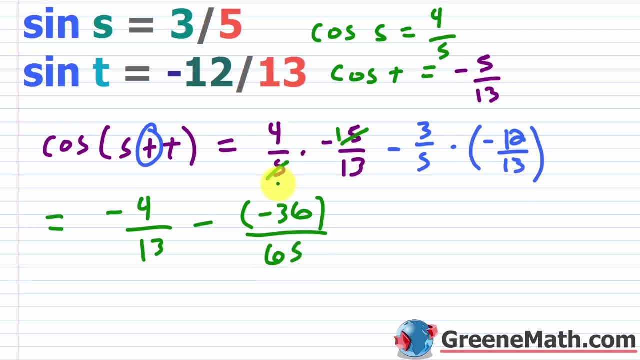 which is going to be 65.. Now I canceled here because we were doing multiplication, but it actually would have been smarter if I wouldn't have canceled, because then I'd have a common denominator. So let's undo this and say: here we have four times negative, five, which is negative. 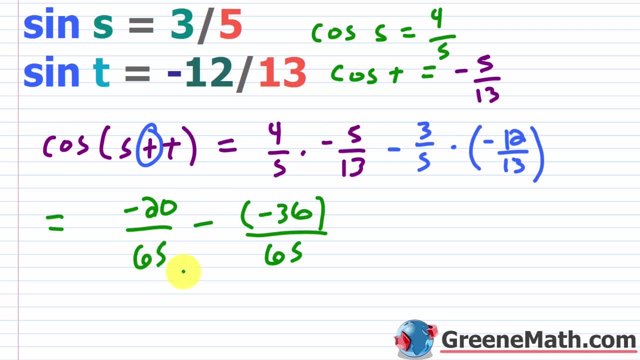 20.. Okay, Over five times 13,, which is 65. In this particular case, it's better to not cancel, because now I have a common denominator and I can basically say what I have: negative 20 minus negative 36.. Again, you've got to be really careful with that sign: Negative 20 minus a. 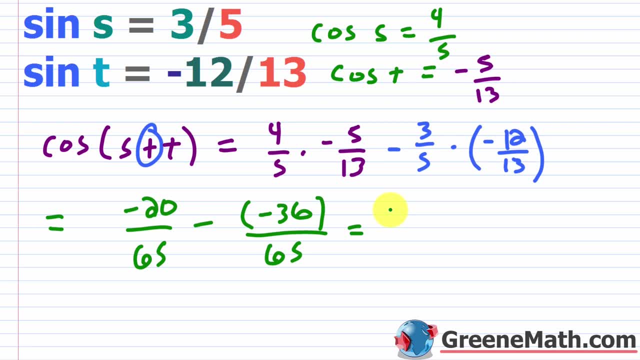 negative 36,, which is going to be negative 20 plus 36,, which is 16.. Okay, Let me write this in different color. So this is going to be 16, and then over you're going to have 65. So this is. 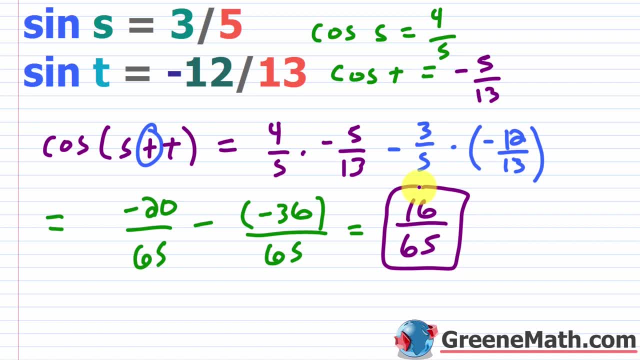 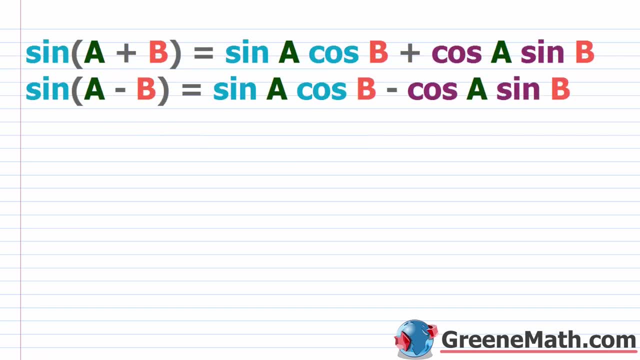 going to be your answer for cosine of s plus t In this lesson we want to talk about the sum and difference identities for sine and also tangent. All right, So we talked about the sum and difference identities for cosine, Now we're just moving on. 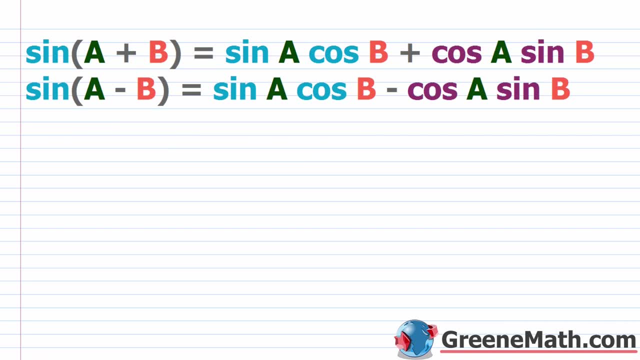 Talking about the sum and difference identities for sine and tangent, Just something you have to memorize. So if we have the sine of, let's say something like a plus b, Again don't distribute that and think it's sine of a plus sine of b. Okay, It doesn't work that way. You have to use 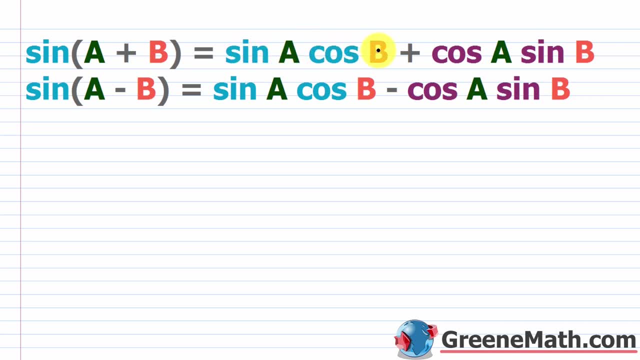 this little formula here. So we're going to say: this is the sine of a times the cosine of b plus the cosine of a times the sine of b. So notice how the sine here and the sine here is the same. Okay, And then, when you get to this one, nothing's going to change except for the sine. So this is a. 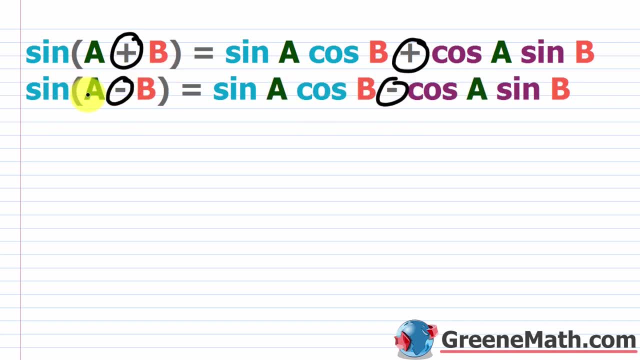 minus and this is a minus. This part right here is the same. So the sine of, let's say a minus b, Now we're going to have the sine of a times the cosine of b minus the cosine of a times the sine of b. So with these you just have to write them down and just go over it a few. 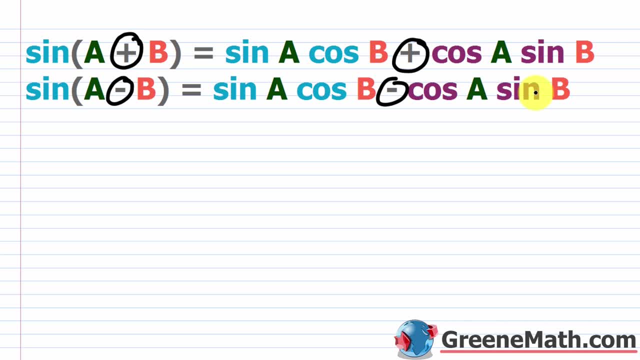 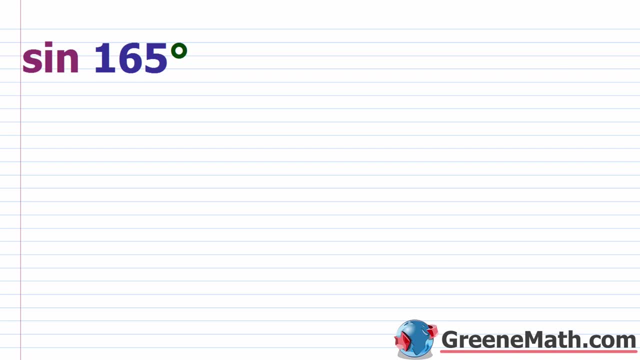 times in your mind, Use it while you're doing the practice and you're going to memorize it. Okay, So let's look at a little sample problem here. You saw this in the last section, where we would basically rewrite something to get an exact value. You're going to do the same thing here, So 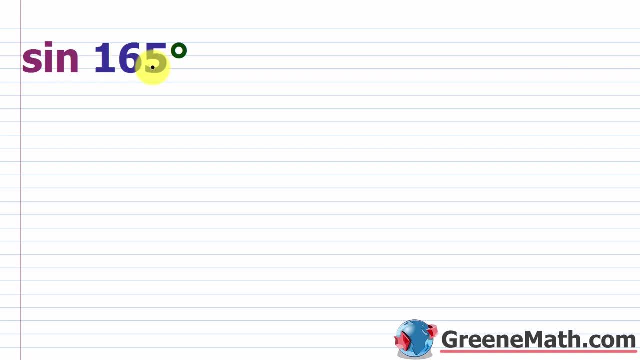 we have sine of 165 degrees. So you're going to find two angles, basically, that are on the unit circle, where you already know things about it. You're going to do the same thing here. So you're going to do the sine of, let's do, 135 degrees plus we're going to go 30 degrees, Okay, So. 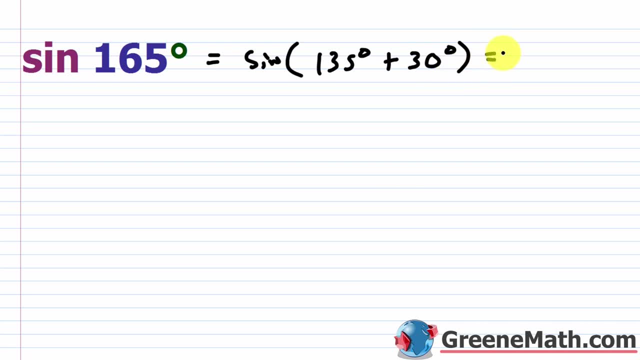 basically, if I use my little sum formula that I just talked about, this is going to end up being what It's going to be: the sine of the first guy. So 135 degrees times the cosine of the second guy, which is the 30 degrees. Then, plus it's the cosine of this first guy, the 135 degrees. 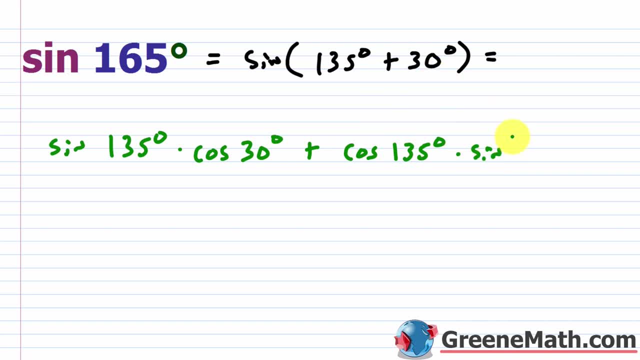 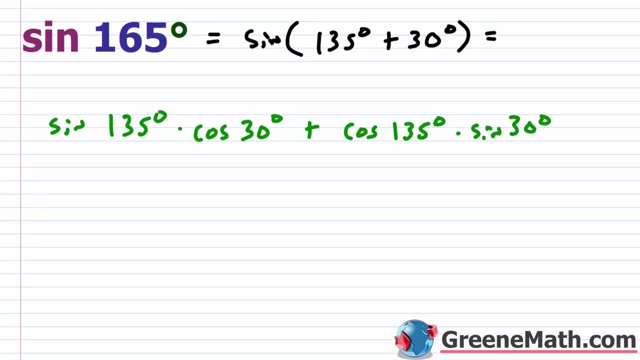 And then, lastly, times the cosine of the second guy, which is the 30 degrees Times the sine of this last guy, the 30 degrees. Okay, So some of you at this point are familiar with the unit circle, others are not, So let's just go really quickly So we can look at this. 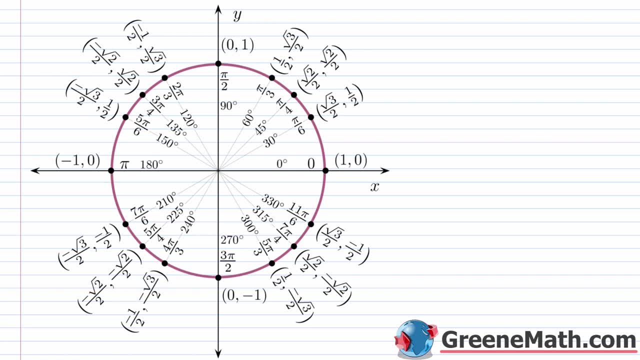 guy, just in case you need to pause the video and we'll get the values. When you're looking at 30 degrees, your cosine is going to be square root of three over two. Your sine is going to be one half Okay. And then, when you look at 135 degrees, your cosine is going to be the negative of the. 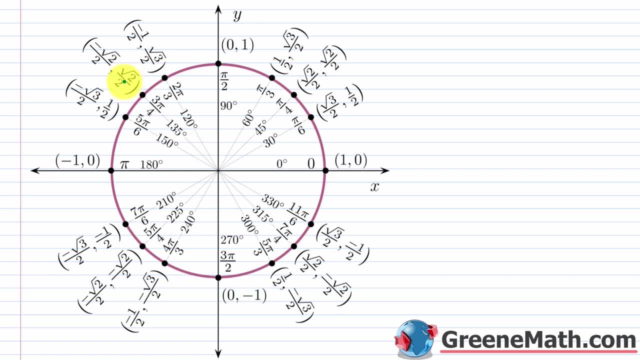 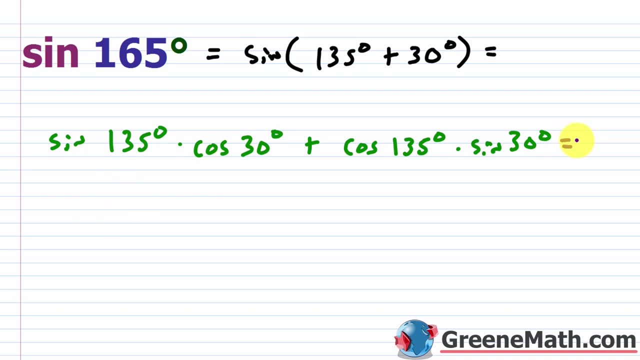 square root of two over two, And your sine is going to be the square root of two over two. So let's come back up And just punch these values in and we'll basically be done. So I'm going to put equals here And then. 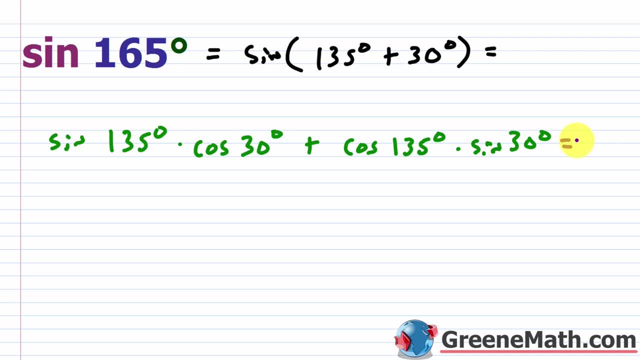 basically, the sine of 135 degrees is the square root of two over two. So I'm going to say this is the square root of two over two times. for the cosine of 30 degrees, I've got the square root of three over two. then, plus for the cosine of 135 degrees, I've got the negative of the square root. 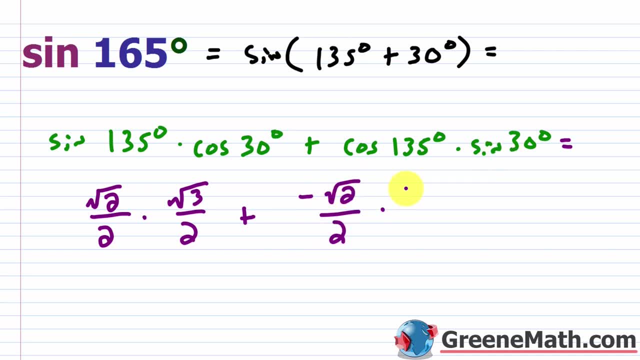 of two over two. And then, lastly, for the sine of 30 degrees, I've got one half Okay. So now all we have left to do here is just basically go through and do some basic operations. So we're going to multiply here. So basically, square root of two times square root of three, really all I can. 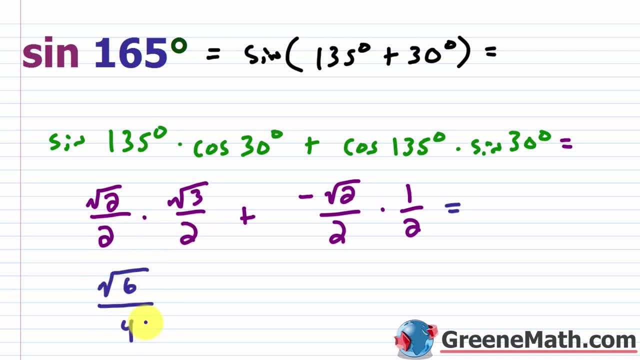 do is say that's the square root of six over two times two, which is four, then plus, if I do the negative of the square root of two times one, it's just the negative of the square root of two. So really I could just change this to minus, okay, and I'll put the square root of two over here over. 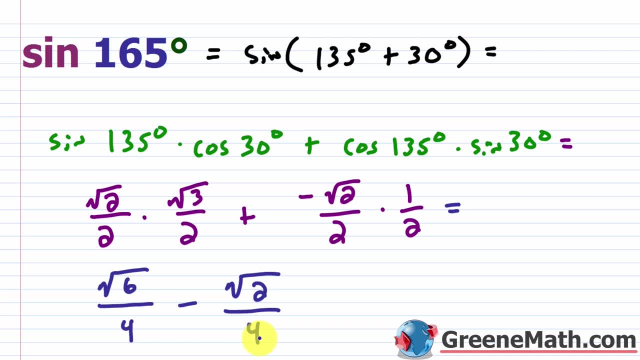 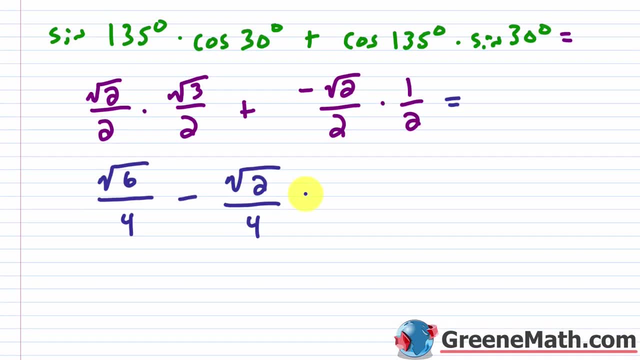 two times two is four. Okay, So basically, in this type of situation, generally speaking, you're going to write this with a common denominator. So I'm just going to come down here, get some room going And I'll just say that this is the square root of six minus the square root of two. 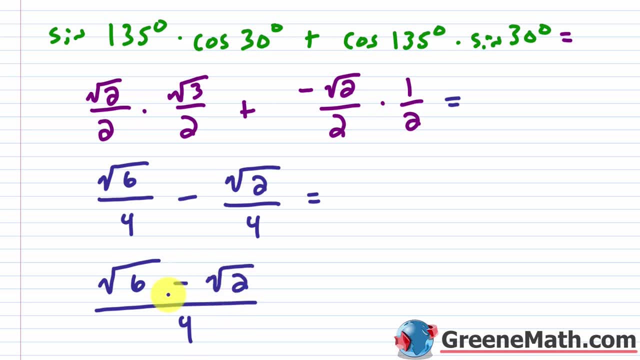 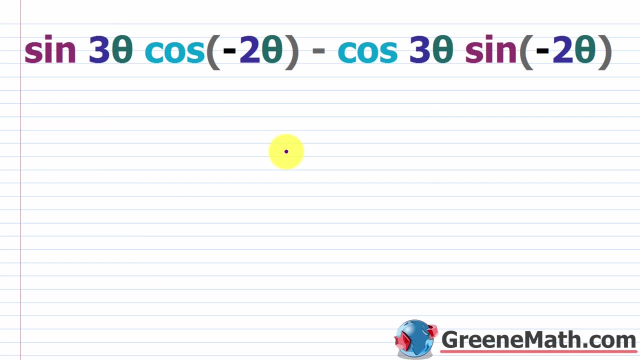 all over the common denominator of four. Okay, so this is the exact value of the sine of 165 degrees. Alright, so another type of problem you'll see is something where you're asked to simplify And basically you just need to realize here that you can use the difference identity for sine. 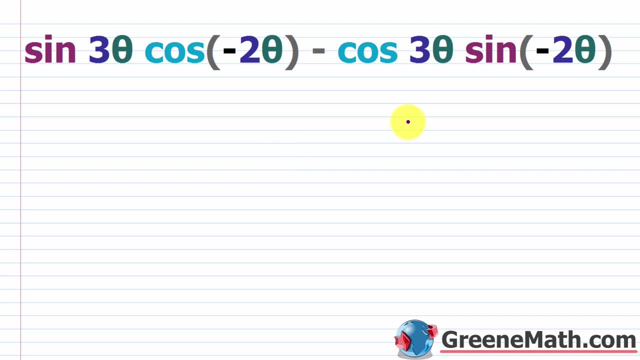 it's kind of going in reverse here, But basically to solve this problem into simplified. So if you notice, here you have sine of three theta times cosine of negative two theta minus the cosine of three theta times the sine of negative two theta. Okay, so if you notice here this angle, 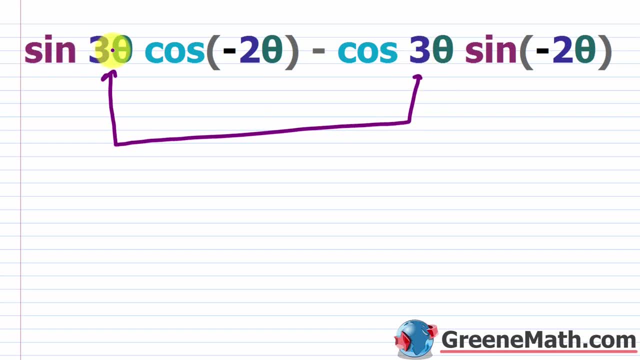 right here and this guy right here. it's the same. you have the sine of this guy and the cosine of this guy and you have a minus. okay, then if you look at this guy, it's negative two theta and negative two theta, cosine of this guy, sine of this guy. So this matches our little formula. 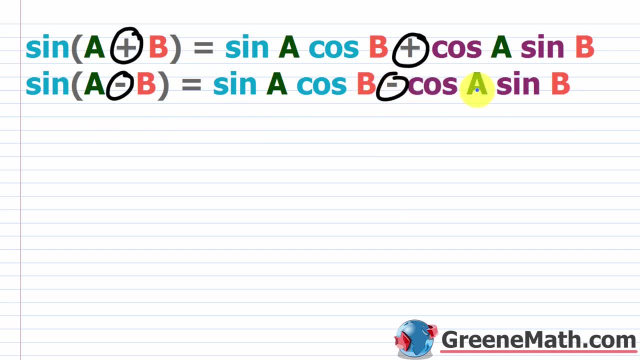 here the sine of A times the cosine of B minus the cosine of A times the sine of B. So in other words, you see sine of three times theta, and then you see the cosine of three times theta over here, And then here you've got this cosine of negative two times theta, okay. And then here you've got. 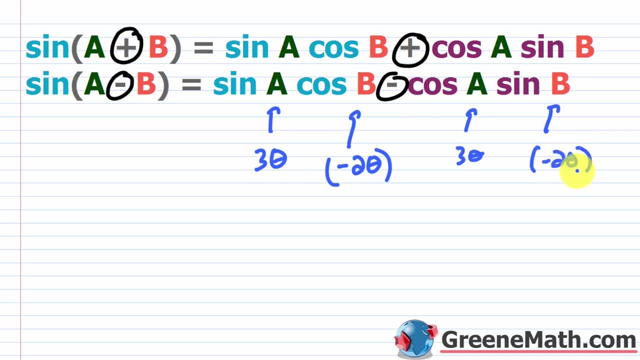 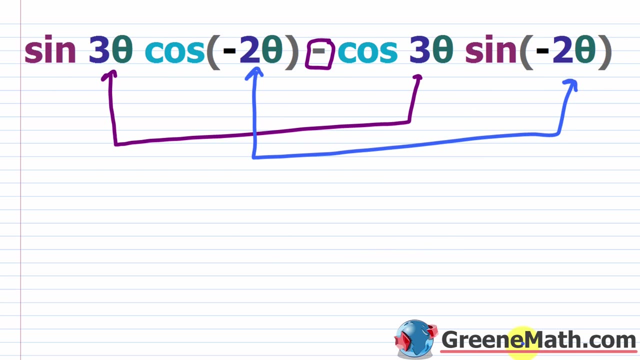 this sine of negative two times theta, okay. So basically, what you're going to do is realize that it's this angle right here minus this angle right here, So it's three times theta minus a negative, which is going to give us five times theta. Okay, so that's what that's going to work out to. So I'll 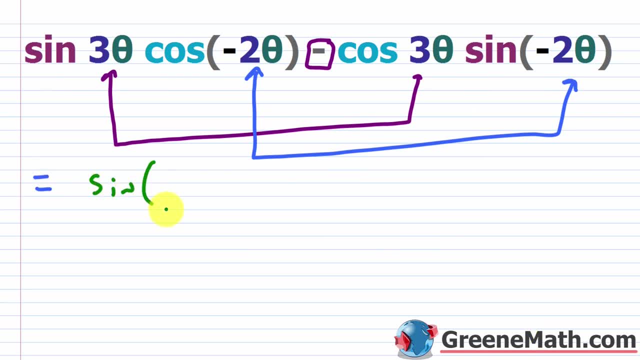 just put equals here. I'm just going to put the sine of- I'm going to take this first angle here- this three times theta minus a negative, okay, you have your two times theta. okay, that guy right there. And so this would give me again, if I just combine this three times theta, basically minus a. 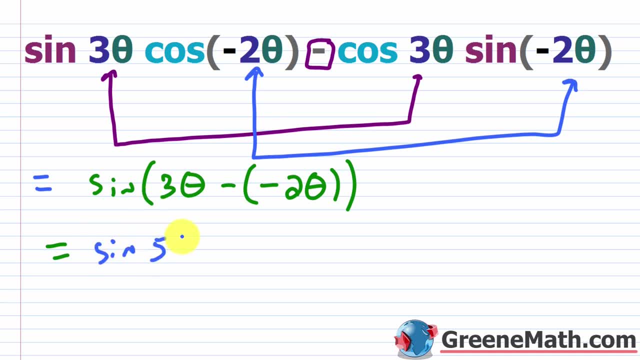 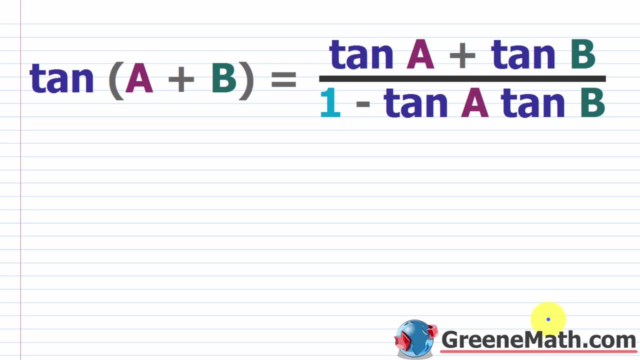 negative is plus a positive, So you would have a sine of five times theta. All right, additionally, we have a tangent, So let's start with the sum guy. So we have the tangent of, let's say, A plus B. this is going to give us: we have the tangent of A plus the tangent of B, over one minus the tangent. 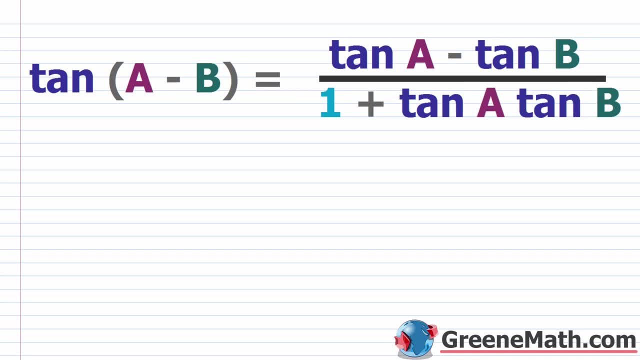 of A times the tangent of B. And what's going to happen when we change over to this difference guy? the signs here just change. So before, with when this was plus, this was plus and this was minus. okay, now that this is minus, this is minus and this is plus. So again, just something you have. 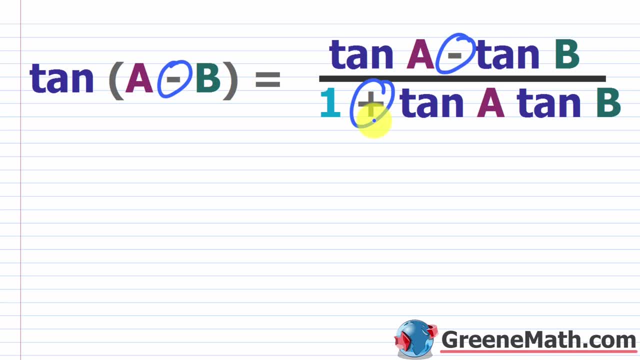 to write down and just keep practicing with, and you will commit it to memory. All right, let's take a sample with this guy. So suppose you're given the tangent of pi over 12.. So if you want to find the exact value again, one way you can do this is by using the sum and difference identities. So I 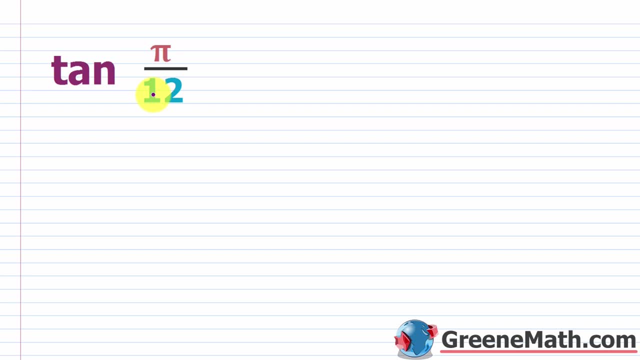 like to work with degrees. when I do this, it's just easier versus me trying to figure out what I need to add or subtract using fractions. So if you can do this with fractions, you know, just skip this step that I'm about to do. But I'm going to convert this first into degrees. 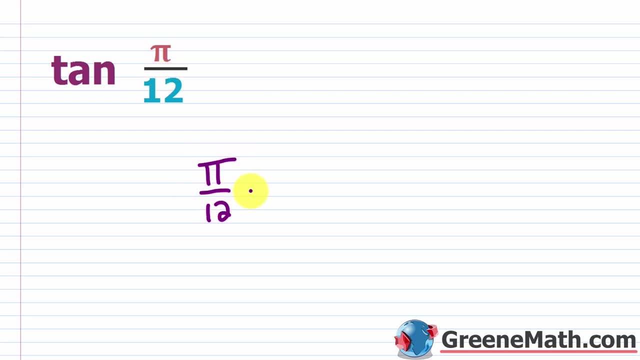 and then you can go back to ratings. Okay, so I'm going to go pi over 12 times, I'm going to go 180 degrees over pi And then basically, this would cancel with this and give me 15 degrees. okay, this is going to cancel out. So pi over 12, in terms of radians, is the same as 15 degrees. 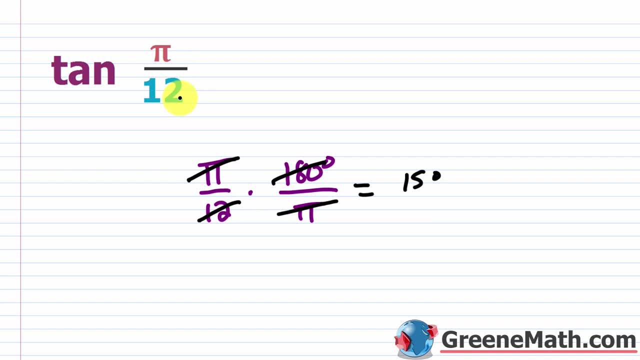 Okay. so now that I got this in terms of degrees, what two angles could I add or subtract to get 15 degrees? Well, one thing you could do is 45 degrees minus 30 degrees. okay, So I could write this as the tangent of 45 degrees in terms of radians is going to be pi over four. 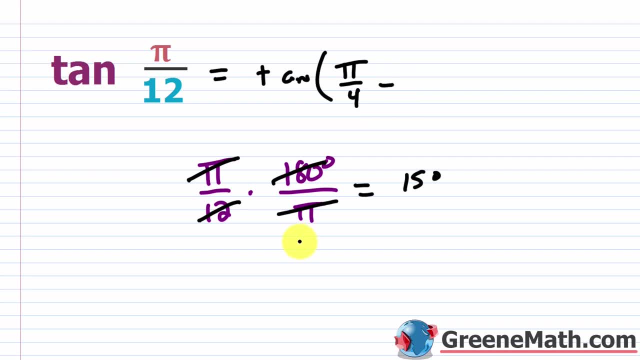 okay, And then minus, if I think about 30 degrees. in terms of radians, it's going to be pi over six. okay, so pi over six, All right. So the next thing I want to do before I even use my formula. 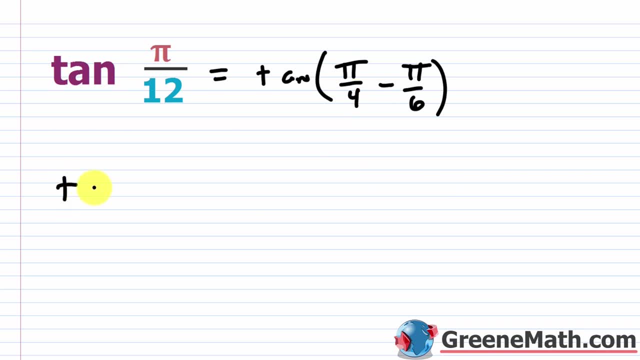 I know I'm going to need the tangent of pi over four. So I know I need the tangent of pi over four And I know I need the tangent of pi over six. Let's go back to the unit circle. I know some of you have this memorized, some don't. So let's just go back to the unit circle. So if we're 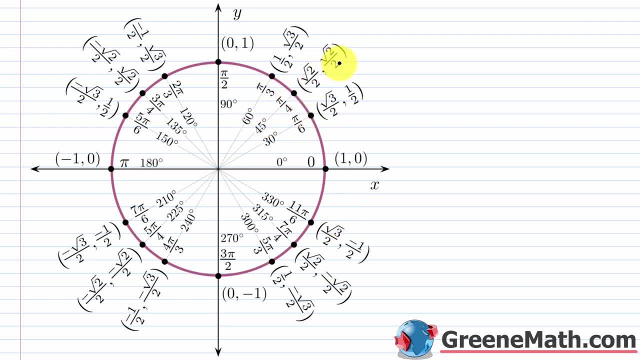 45 degrees, we have square root of two over two and square root of two over two. So that means the cosine and the sine are the same And basically the tangent is the sine divided by the cosine. And since it's the same number, right same number divided by itself is going to give you: 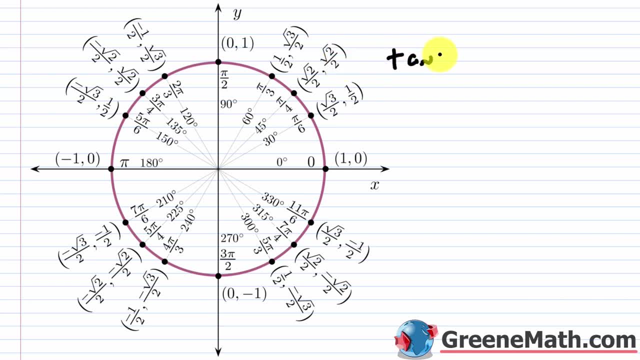 one. Okay, so we know that. I'll just write this down. the tangent of pi over four is just going to be one. okay, because you have square root of two over two divided by square root of two over two, So that gives you one. then the tangent, if I think about four, pi over six, this is going to be. 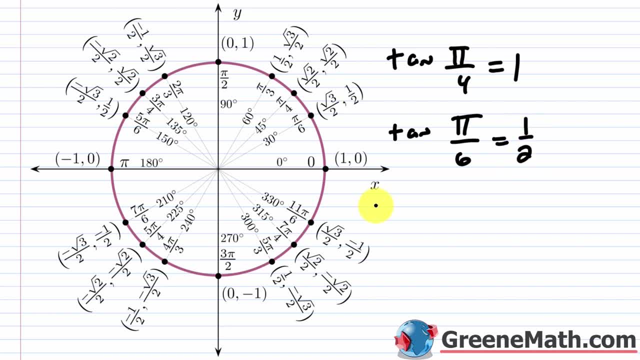 one want the sine, which is one half divided by the cosine, which is a square root of three over two. So basically I would flip this guy, okay, because I'm dividing fractions. So let's put the two up here and the square root of three over here, okay, And then basically the twos cancel and I 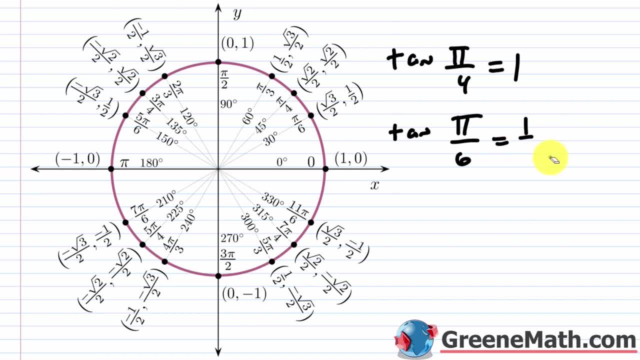 have one over the square root of three, So one over the square root of three. of course, we're going to rationalize this, So I'm going to multiply this by the square root of three over the square root of three, And so this is going to give me the square root of three over three. Okay, so let me. 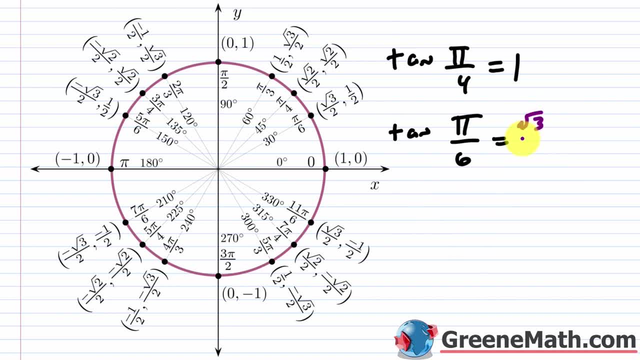 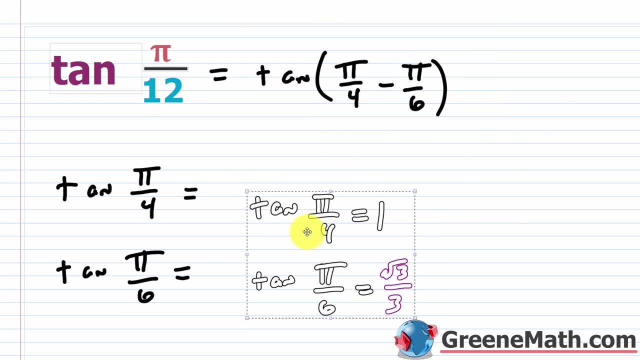 write this in a more compact way. So square root of three over three. let's copy this, okay, And let's go back And let's just paste this in here real quick, And so this is one, this is one, and 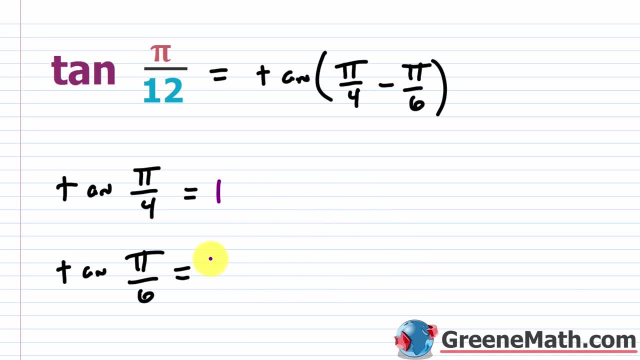 this is square root of three over three. Okay, so, square root of three. square root of three over three. Okay, so now that we figured that out, we can use our little difference identity And for this guy right here, let me put equals. it's going to be- I'm just going to slide this off to the 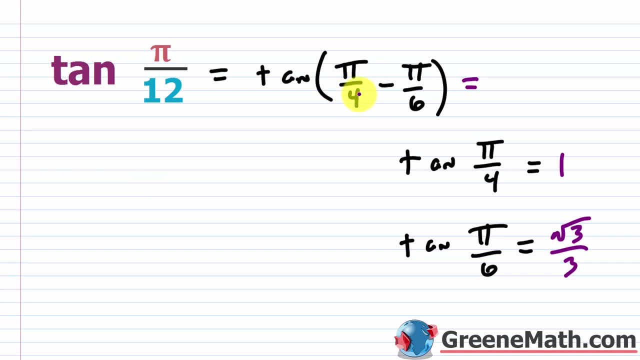 side for one second. So this is going to be the tangent of the first guy. So the tangent of pi over four is going to be one. So it's going to be one then, minus the tangent of the second guy. So minus the tangent of pi over six, which is the. 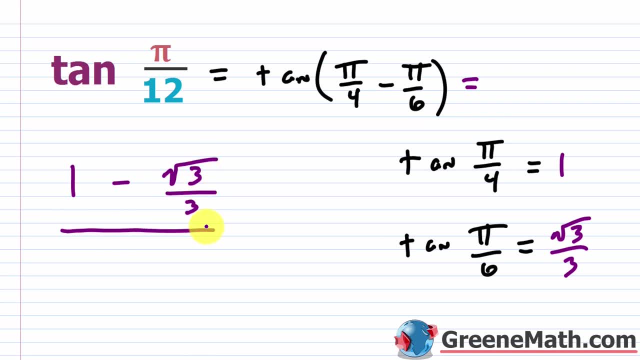 square root of three over three. then this is over. remember, you have your one. the sign is different here, So it's going to be plus, you're going to multiply them together, right? So the tangent of pi over four times the tangent of pi over six, So basically one times this guy. So it'd 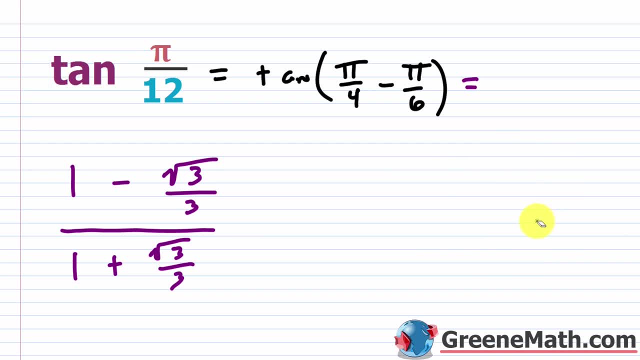 be minus. we don't need it anymore Now, basically, you have a lot of different options here. when it comes to simplifying, Okay, I am going to choose to basically multiply the numerator and denominator of this guy by three, Okay, so this is going to get distributed here and here this is going to. 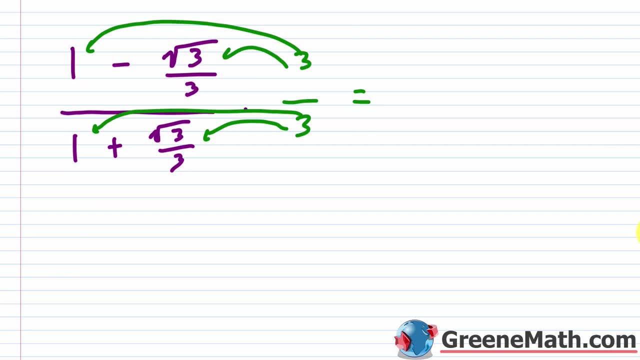 get distributed here and here. So what is this going to give me? Let me scroll down and get some room going. So three times one is obviously three, and then minus this would cancel with this and I'd have the square root of three there. Okay, so we'll put this over here and I'll kind of undo. 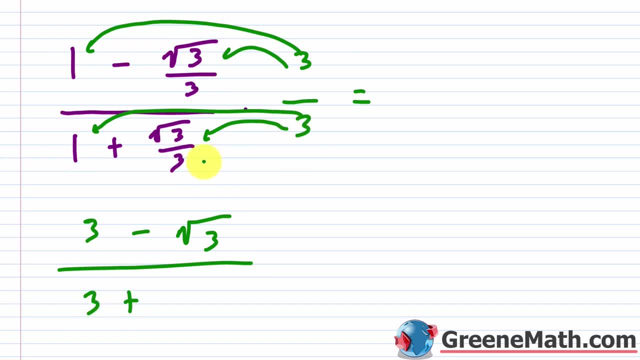 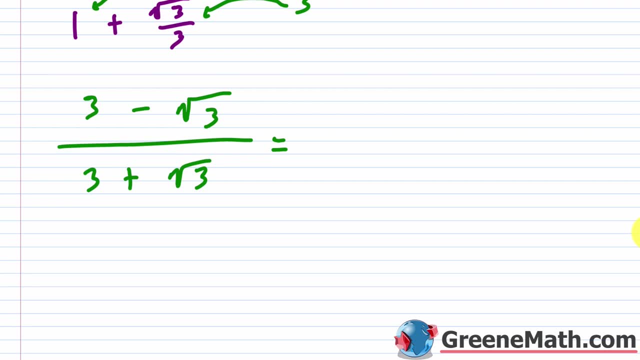 over here. three times one is three. then plus again, the threes would cancel there and you'd have the square root of three. Okay, so now this is a little bit simpler, But really, in order to go anywhere, what I'm going to do, remember, if you have a radical down here, you have this plus. 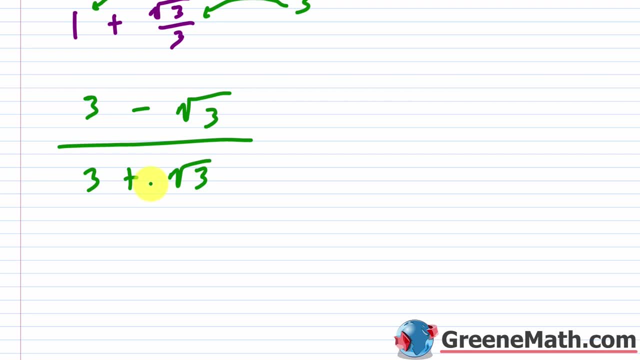 here. this is binomial, like this. then basically, what you can do is you can multiply by the conjugate. Okay, so I can wrap this and I can wrap this. So I'm going to multiply this by. I'm going to have three minus. okay, I'm changing the sign from plus to minus. then the square root of three: 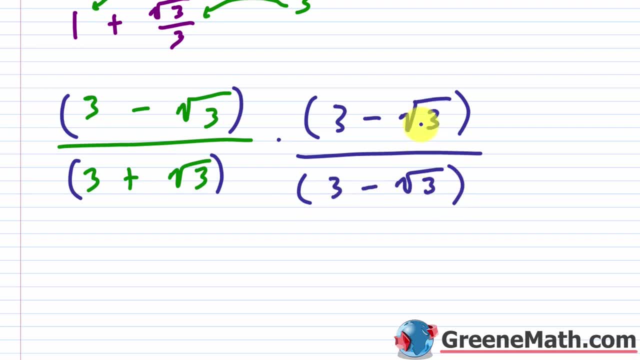 then over you would have three minus the square root of three. Again, this is just a complex form of one. When you multiply these guys together, you're just going to do the first guy squared minus the last guy squared. Remember the middle? two guys are going to drop out. Okay, so let me 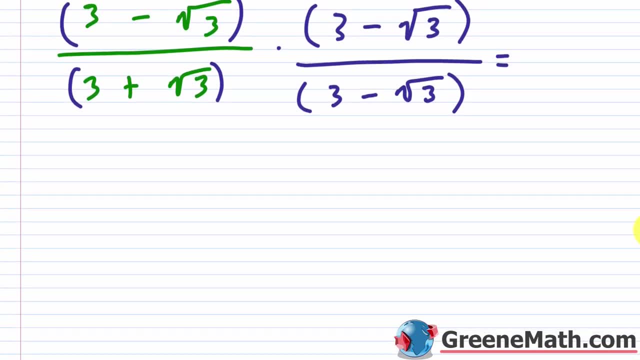 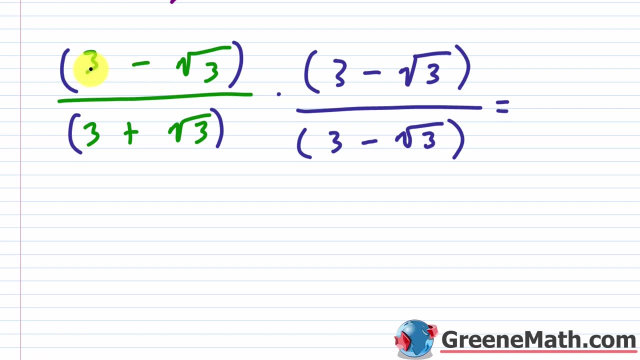 make sure I got my equal sign going, So put that in there. Let's keep going. All right, so in the top, realize this is three minus square root of three, quantity squared. So I can use a formula on that: Take the first guy and square it, So three squared, and then this is minus, So minus it's. 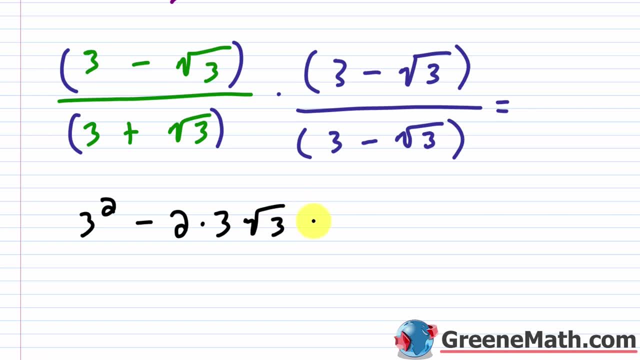 three times the last guy, which is three times the last guy, which is square root of three, And then plus the last guy, squared of three squared is three. Okay, you can simplify this right now: Three squared is nine. Then, basically, two times three, you know that's six. you'd have minus six times. 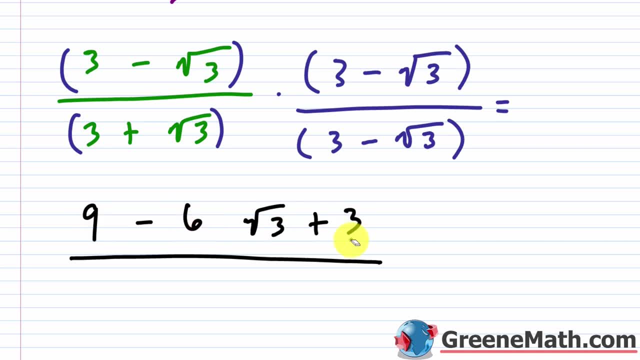 square root of three, and then plus three. Now nine plus three is 12.. So let me just go ahead and put this as 12 minus six times the square root of three. Okay, so we have that, And I can even shorten this a little bit and put this like this: Now down here, all I need to do is square. 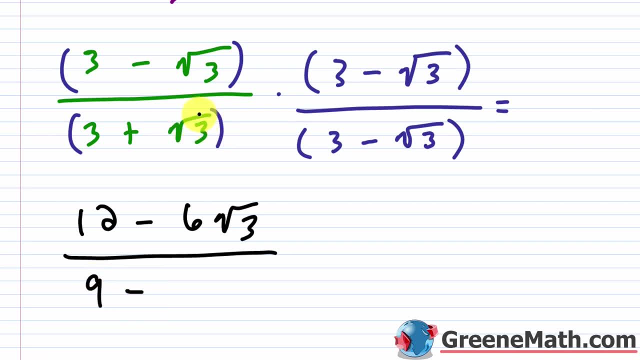 is nine and then subtract away. If I square this guy, square, root of three squared is just three. Now I can just perform this operation: nine minus three is just six. Okay, Now we're not done, because notice that you have 12 here, which is divisible by six, six here, which is divisible. 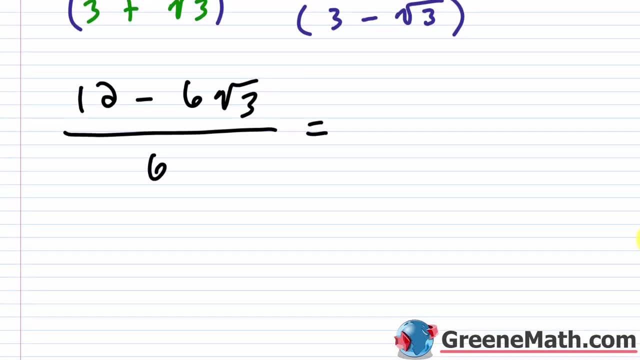 by six and six here. Okay, so what I'm going to do is I'm just going to factor. I'm going to factor a six out from the numerator. So this is going to be two minus the square root of three, okay. 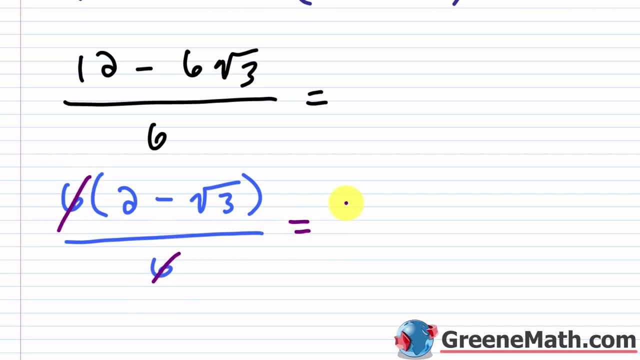 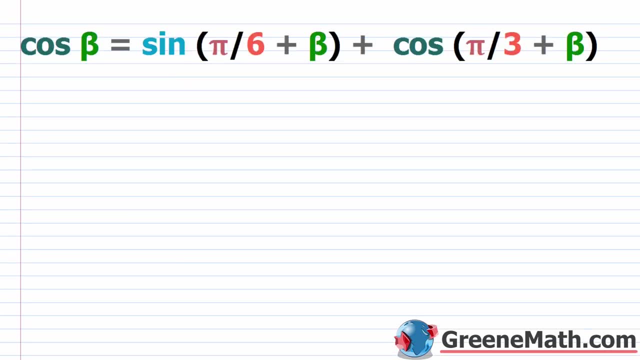 over six down here. And now we're done. right, we cancel this and I end up with two minus the square root of three as my answer for the tangent of pi over 12.. All right, let's look at an example where we're going to verify an identity. So we have: the cosine of beta is equal to the sine. 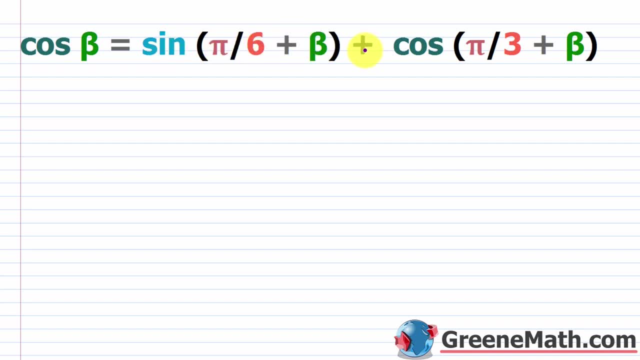 of we have this pi over six plus beta, and then plus we have cosine of we have pi over three plus beta. Okay, so basically we always want to work on the more complex side. Obviously, the right side is way more complex, So I'm just going to put equals over here. Okay, normally we line this up. 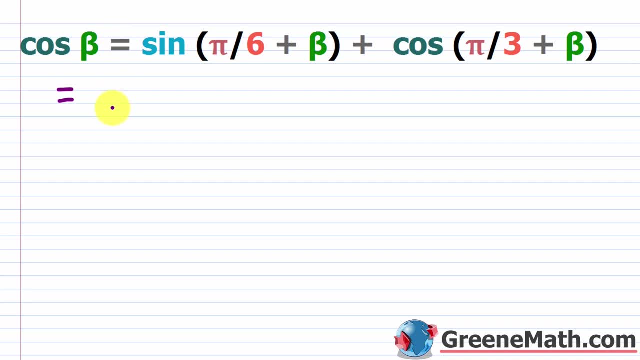 but I want to give myself lots of time, So I'm just going to put equals over here, Okay and so basically, what I'm going to do is I'm going to use my sum identity here and my sum identity here. Okay, so I'm going to first say that I have the sine of this pi over six times the cosine of. 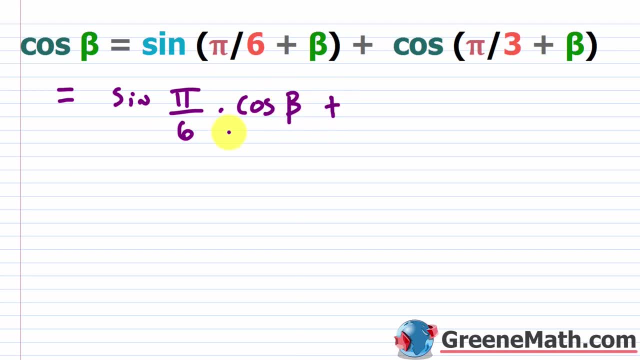 this beta. okay, then, plus okay. so now I'm going to do the cosine of this guy right here. So let me change color. So I'm going to go the cosine of this, in this case pi over six and then times. 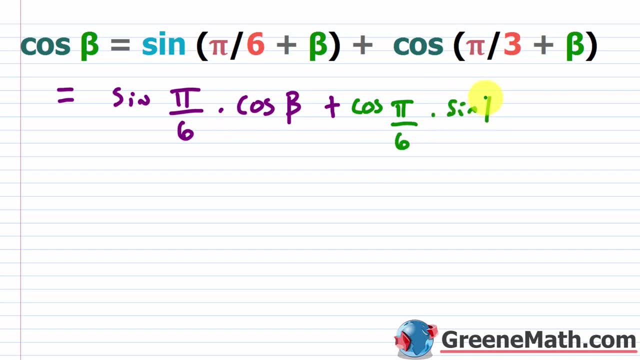 you have your sine of beta, so your sine. Now, additionally, I want to do the same thing with this cosine guy, So I'm going to put plus here. Remember how to do this. I'm going to go cosine of this guy, So cosine of pi over three. 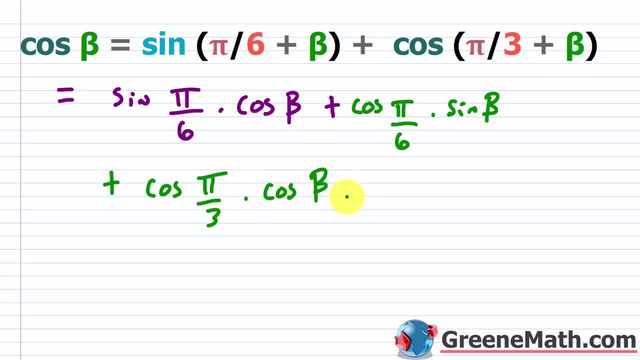 and then times the cosine of the next guy, So cosine of this beta here, And then if this is plus, it's going to go minus, right, so the signs are going to be different there. And then now I'm going to do the sine of this guy, sine of pi, over three times the sine of beta. Okay, so now what? 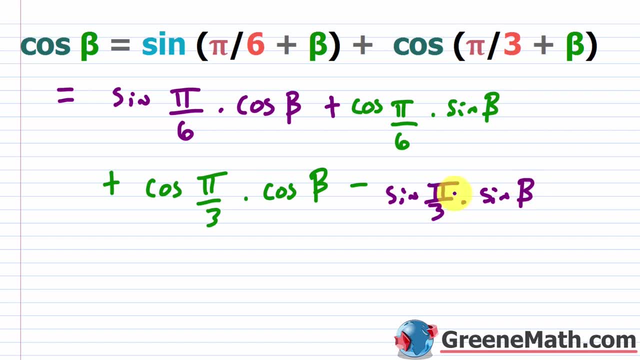 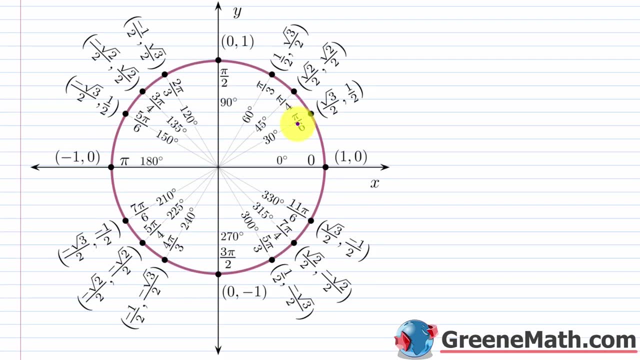 we want to do is we want to do the cosine of this guy, sine of pi over three times the sine of beta want to do is think about what can we replace. Well, think about the fact that you have the sine of pi over six and the cosine of pi over six. So, coming back to my unit circle, again, we think 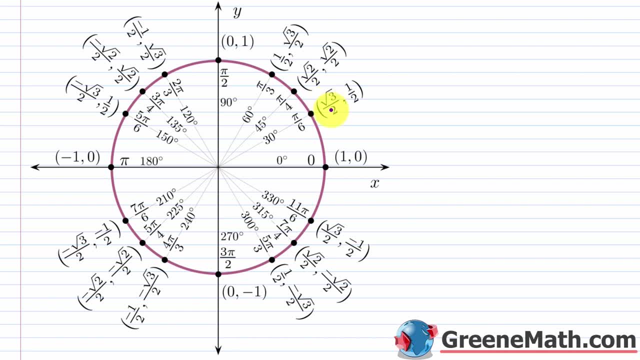 about pi over six. the sine is a half and the cosine is square root of three over two. So let's just write this down. So we have the sine of pi over six is one half And we had the cosine of pi over six. that's going to be the square root of three over two. Now, additionally, we're also: 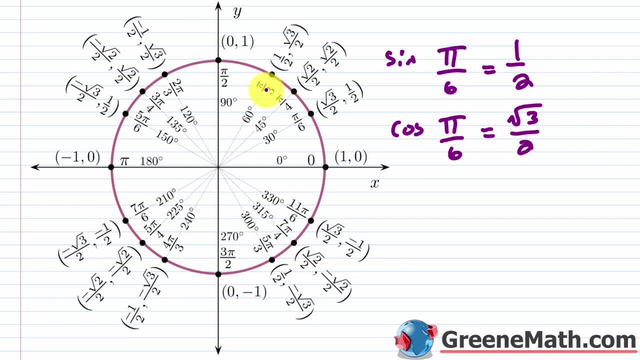 working with this pi over three, right? So we're going to do the cosine of pi over six and then we need the sine and cosine for that guy as well. Okay, so the cosine for pi over three is going to be one half and the sine for pi over three is going to be the square root of three over two. 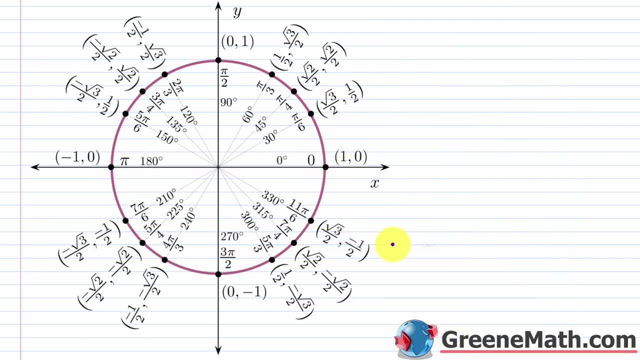 Okay, so let's go ahead and grab this guy And we're going to cut it away, And I'm just going to come down here real quick and paste this in, So we have it. So let's just replace the sine of. 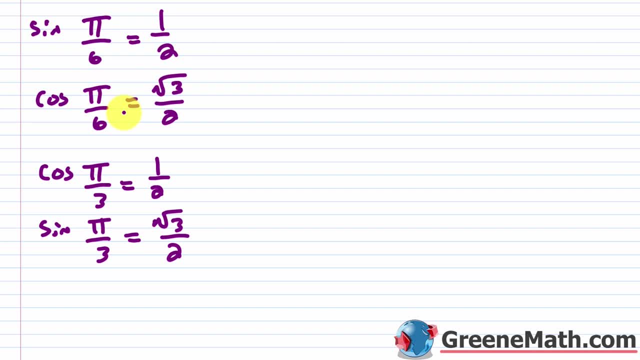 pi over six with one half and the cosine of pi over six with square root of three over two. Okay so, let's come up here. So let's go ahead. I'm going to put equals. instead of the sine of pi over six, I'm going to put one half. 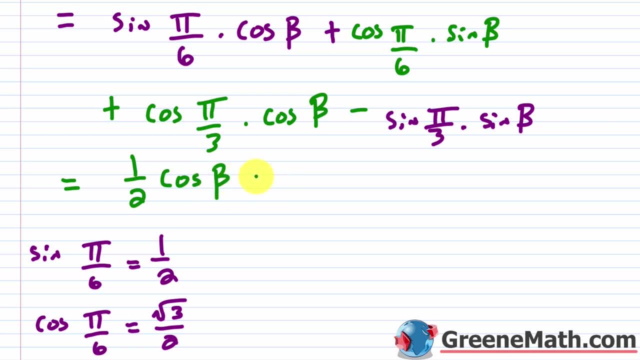 and then times my cosine of beta, Okay. Plus, for this guy right here, I'm going to put the square root of three over two, So the square root of three over two times my sine of beta, Okay. And so let's get rid of these two right here. we don't need them anymore. And let me scroll down a little. 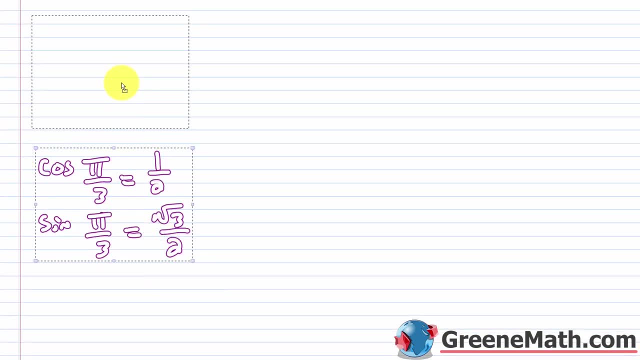 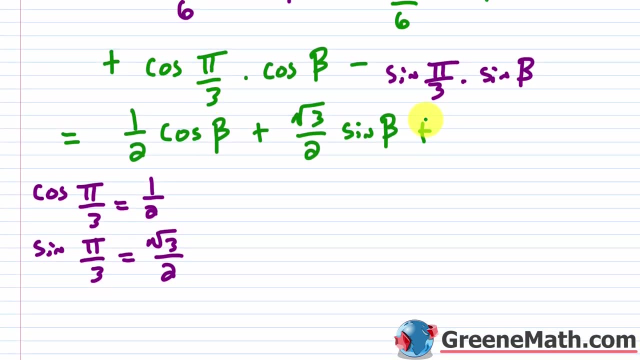 bit And I'll drag these up into our visual range. Okay, so we can work with them. Let's come back up here real quick. Okay, so I'm going to replace this cosine of pi over three, So I'm going to put plus. 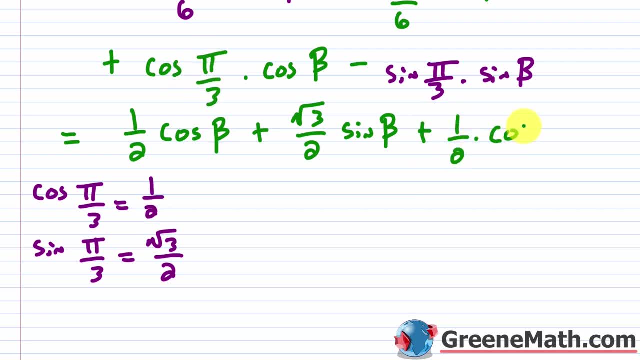 this guy is going to be one half and then times your cosine of beta. Okay, so let's get rid of this. And then, lastly, I'm going to put this minus. here we have the sine of pi over three, which is the square root of three over two. So let's get rid of this. And this is times our sine. 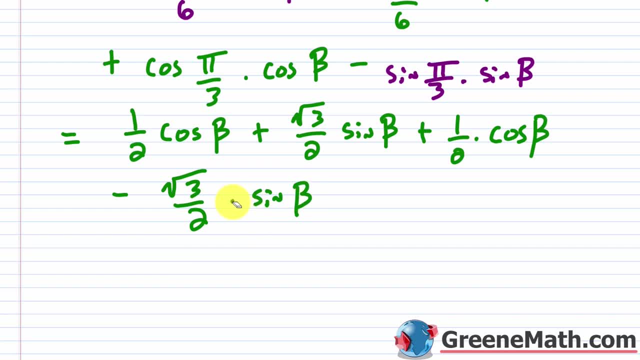 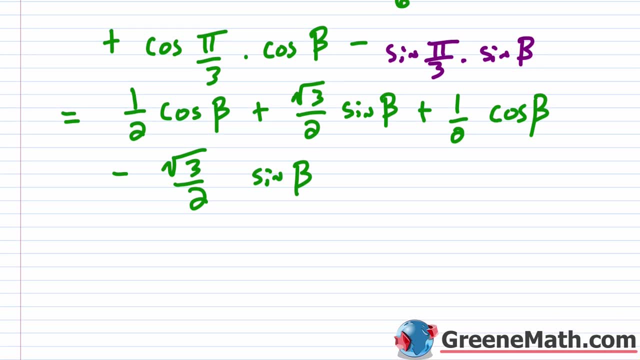 of beta, Okay, And sometimes I put multiplication signs and sometimes I don't. you don't need it, Sometimes I just put it there, Okay. so let's scroll down a little bit. a little bit more room going, let's think about what we can do. So we'll notice here that this guy 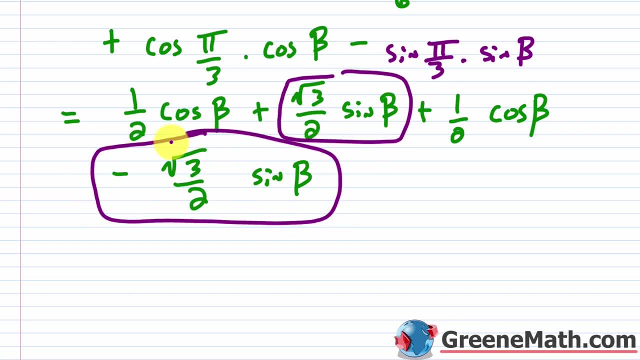 right here. okay, and this guy right here, those can be canceled, right? You have the square root of three over two times the sine of beta, And then you have the negative of that, So I can just cross that out. those are gone. So basically I can say this is one half times cosine of beta plus one. 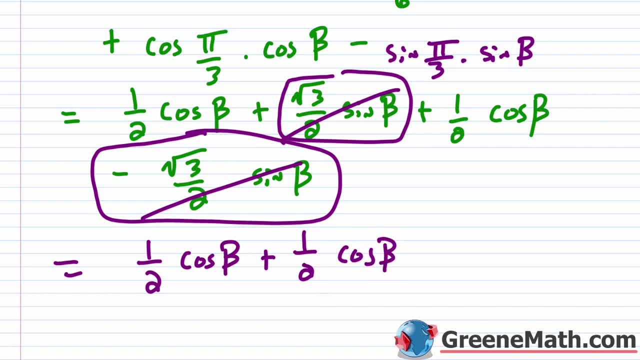 half times cosine of beta. So let's stop for a second. Remember what we're trying to get. we're trying to just get the cosine of beta. So basically, if you have a half of something plus another half of something, you're going to get the cosine of beta. So let's stop for a second. 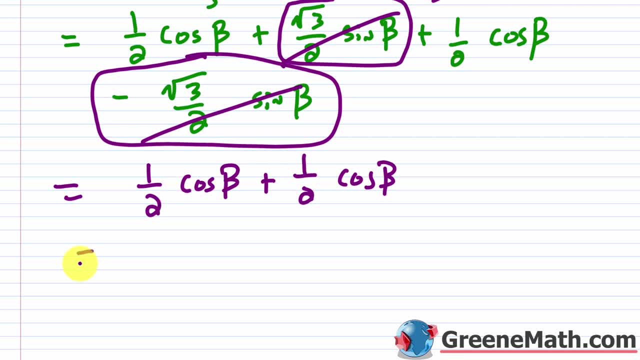 If you have another half of something, you have one of that thing. you basically have a common denominator here, right? you could say: this is the cosine of beta plus the cosine of beta over two, right, and you have two of this. So let's go ahead and come down here and just say that we have. 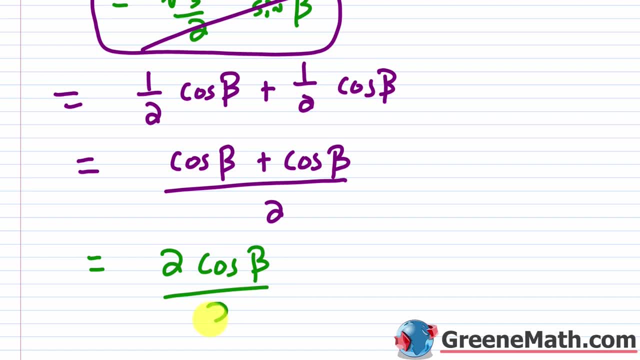 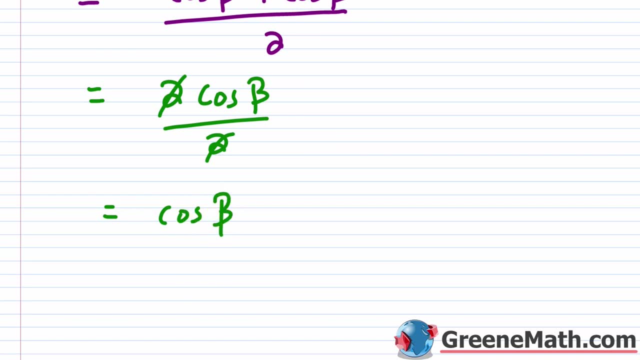 basically, two times the cosine of beta, over two, we can cancel that And, lastly, we will say that we have the cosine of beta. Okay, And so we verified our identity. All right, let's look at one other type of problem. here we're going to be asking ourselves: what is the cosine of beta? 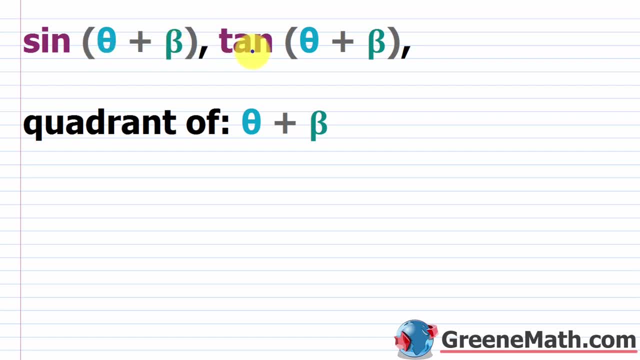 We're going to ask to find the sine of theta plus beta, the tangent of theta plus beta and the quadrant of theta plus beta. So a very common type of problem. Unfortunately, they do take a while to work out. So let's go ahead and come down here, And for this one, I'd like for you to try it on. 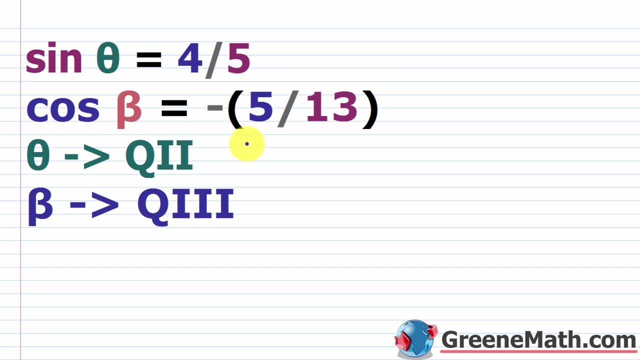 your own before we even go. we did a similar problem with cosine in the last lesson. So we have sine of theta is equal to four fifths. we have the cosine of beta, which is equal to the negative of five thirteenths, And then we're told that theta is in quadrant two. 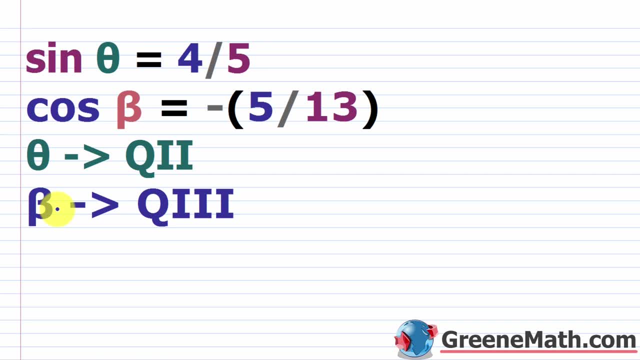 and beta is in quadrant three, Okay. So how do we figure this out? Well, what we need is the cosine of theta, So that equals what. Okay, that equals what. And we need the sine of beta, So that equals what. Okay, if we have these two pieces of information, 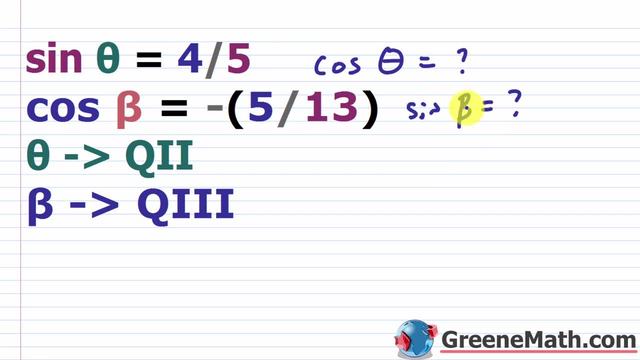 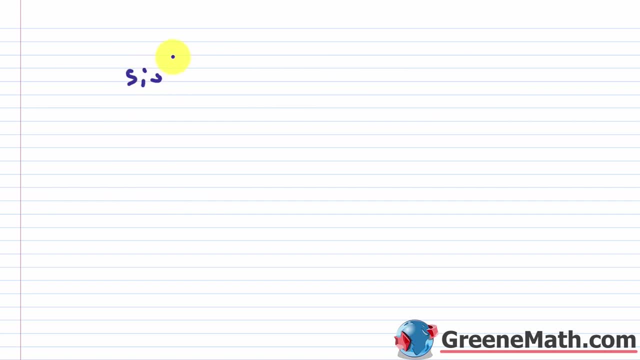 then we can use our little formulas that we've been talking about in the lesson. Okay, So, basically, how do we get this If we know the sine of theta is four fifths? Well, I can start off by saying: well, the sine squared theta. 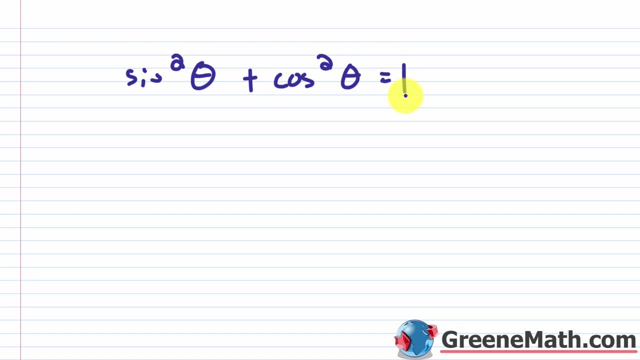 plus the cosine squared theta equals one. okay, remember your Pythagorean identity, So I can plug in here a four fifths And that's going to be squared right. So four fifths and this is going to be squared, So this ends up being 16 over 25, plus the cosine squared theta. 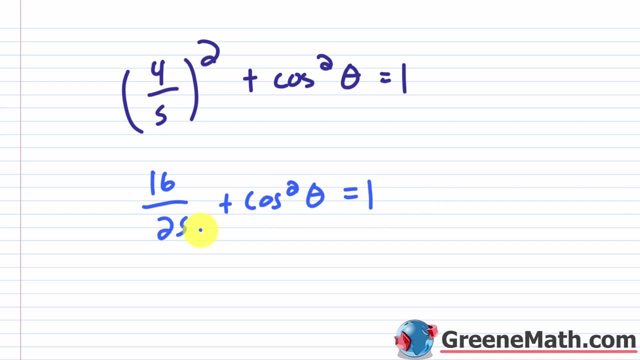 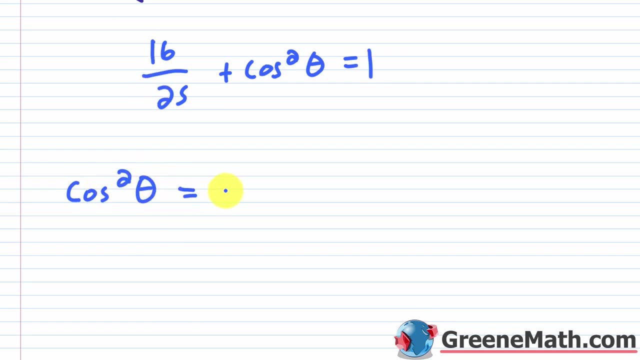 is equal to one. Again, I'm just going to move this over here, So let me scroll down a little bit. I'm just going to say that I have cosine squared theta is equal to if I subtract this over 25.. If I make this as 25 over 25, then basically 25 minus 16 is nine. so you would have. 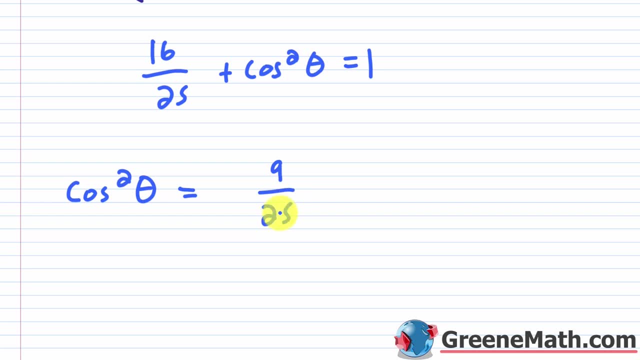 nine, twenty, fifths, Okay, But now the issue is: I want cosine of theta, not cosine squared theta. So basically, I need to square root each side- Remember you get plus or minus over here- And then, based on what quadrant you're in, that's how you decide what sign you're going to use. 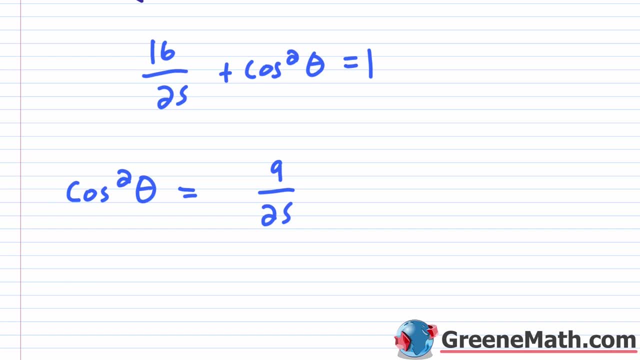 Now we're told that theta is in quadrant two. okay, and in quadrant two cosine is negative. So I'm going to go. cosine of theta is equal to. I'm going to use the negative of the square root of nine over 25.. 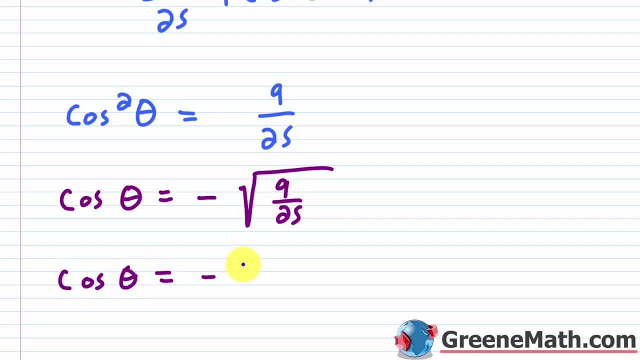 And of course, this is going to end up giving me. the cosine of theta is equal to negative. square root of nine is three, and then the square root of 25 is five, So negative three fifths. Okay, So let's take this up. So we're just going to cut this away And actually I'll just write: 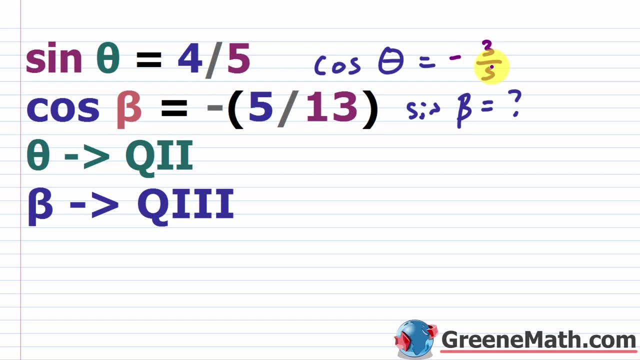 it in here. So I'll put negative three fifths. So that's the first piece of the puzzle. So now we need to find the sine of beta. I'm going to use the same thought process. So the cosine of beta is five thirteenths. So again we have the sine squared, in this case beta plus cosine squared. 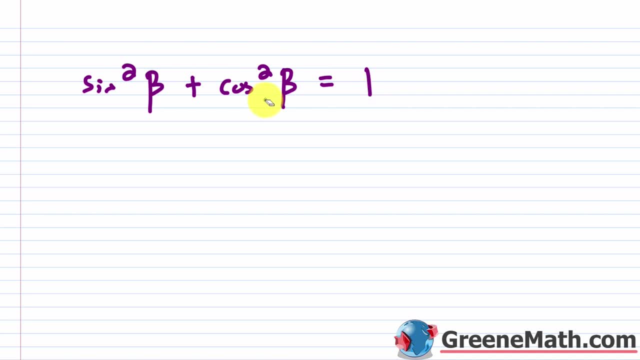 beta is equal to one. And for cosine squared beta, remember for cosine itself. I'm plugging in a negative five thirteenths and this guy's being squared. Don't forget to square. Okay. So if I square this guy, I'm going to get 25 over 169.. So I'm going to have sine squared beta plus this guy. 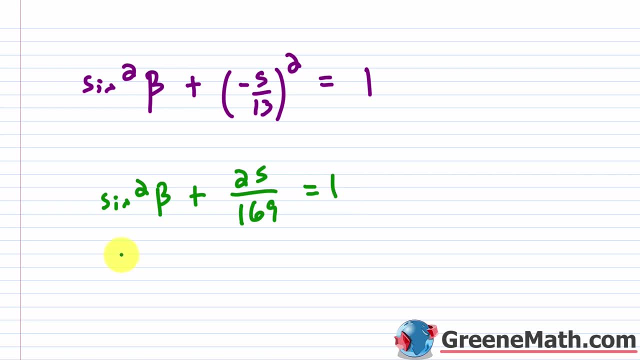 here equals one Same thing. I'm just going to move it to the other side. So I'm going to have the other side. So I'm going to say: sine squared beta is equal to. let me go ahead and put this as a common denominator. So 169 over 169, same thing as one. then minus this guy over here, just moving. 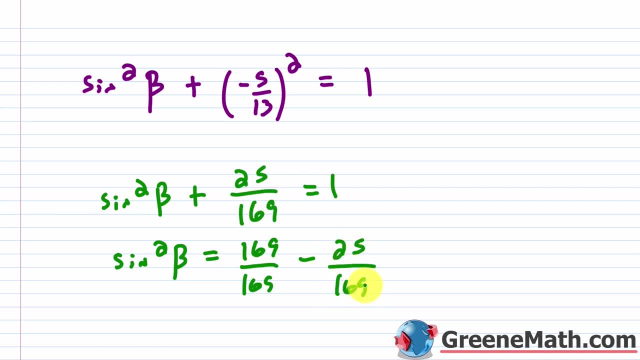 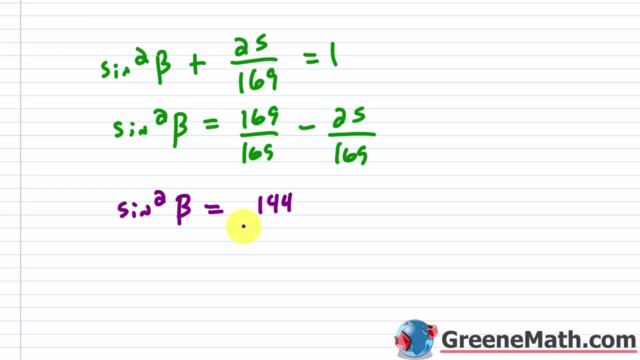 to the other side. So minus your 25 over 169.. And so the sine squared of beta is equal to 169. minus 25 is 144.. So you have 144 over 169.. Now we said that beta was in quadrant three and in quadrant. 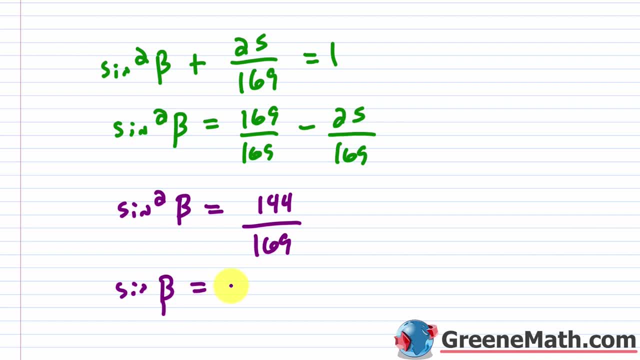 four, we said that the sine squared of beta is equal to the negative of the square root of this guy, So the 144 over 169.. So the square root of 144 is 12.. The square root of 169 is 13.. So I'll go. 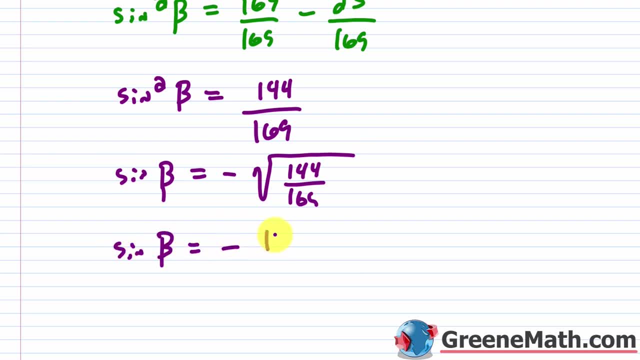 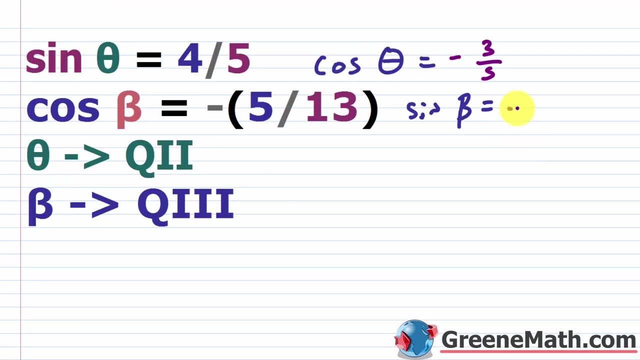 ahead and say: the sine of beta is equal to the negative of 12 thirteenths. Okay, So the negative of 12 thirteenths. So let's put this up here: the negative of 12 thirteenths. Okay, So we are. 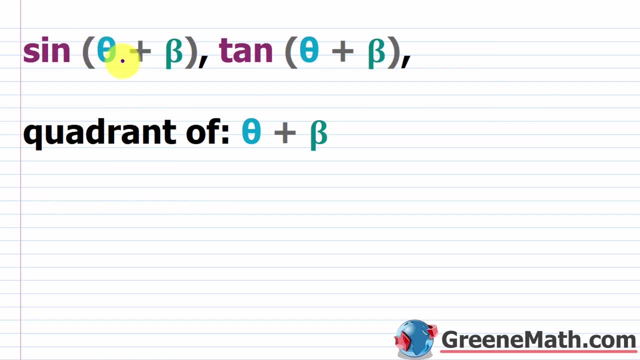 officially ready to answer this part up here. the sine of theta plus sine squared, So I'm going to plus beta. Okay, So basically you would have: the sine of theta plus beta is equal to the sine of theta, which is four fifths, multiplied by the cosine of beta, which is negative five thirteenths. 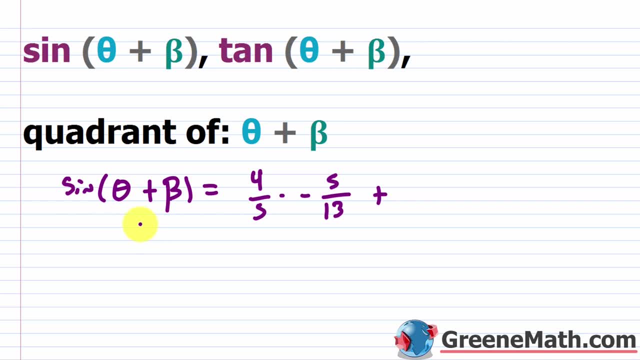 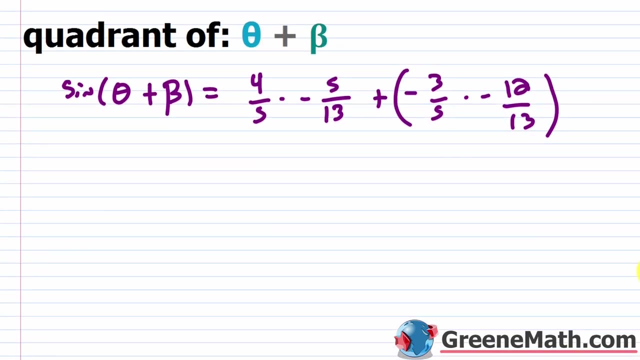 Okay, Then plus, you have your cosine of theta, which is negative three fifths, and then times your sine of beta, which is negative 12 thirteenths. Okay, I'm going to wrap this in parentheses so I don't make a silly sign mistake. Now, in a lot of cases you'll notice. 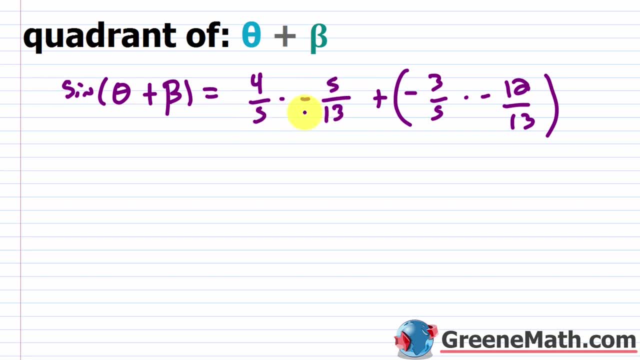 when you're multiplying here, you can cross cancel Here. notice that you have five times 13 and five times 13.. So don't cancel this because you're going to want to have a common denominator. I make that mistake all the time, So I'm just going to stop you from doing it, Okay? So basically, 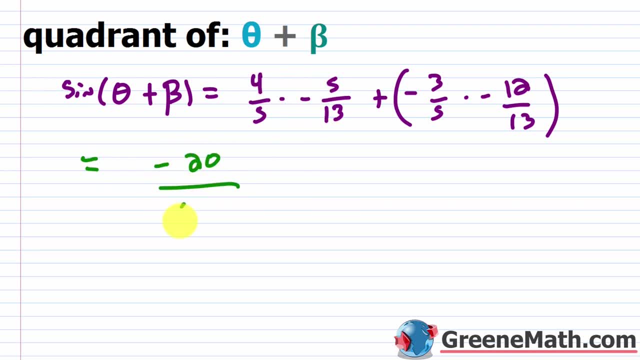 four times negative five is negative 20.. This is over Five times 13, is 65. Then, plus negative times negative is positive. So three times 12 is 36.. Over five times 13 is again 65.. Okay, So to finish this up, I'd have negative 20 plus 36,, which is 16,, and then over the common 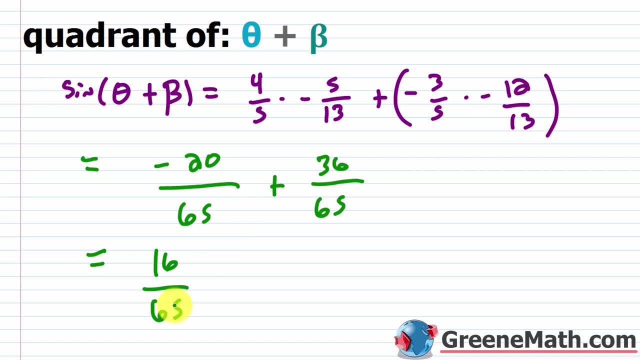 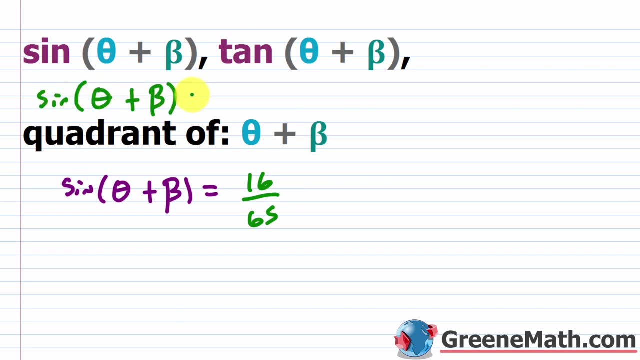 denominator of 65. So sine of theta plus beta is 16 over 65. So let's just erase all this work. So sine of theta plus beta is equal to 16 over 65.. Okay, So how do we get the tangent of theta? 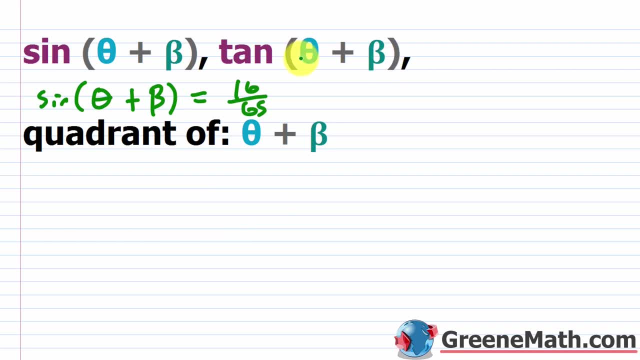 plus beta. Well, first I need the tangent of theta and I also need the tangent of beta. So how do I get that? Remember, for the tangent, I divide the sine by the cosine. So if I think about, let me go down here because we're going- 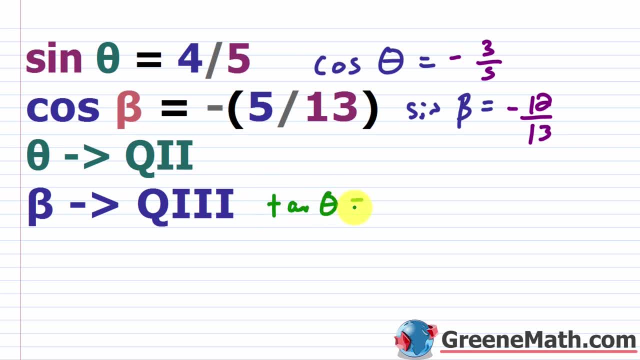 to forget stuff. So if I want the tangent of theta, it's going to be the sine of theta, which is four-fifths. So four-fifths divided by the cosine of theta, which is negative, three-fifths. Again, we're dividing fractions. So flip this guy. I'm going to multiply by the reciprocal So times. 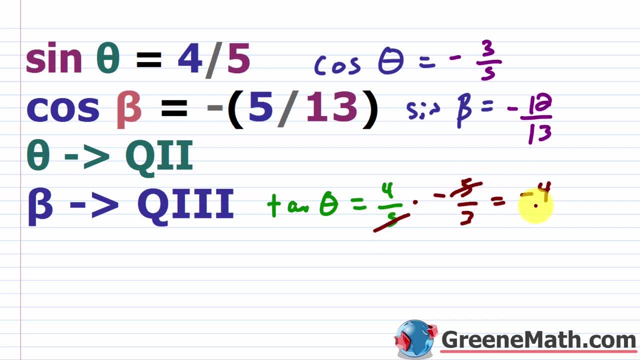 five-thirds. This cancels and I get negative four-thirds. Okay, So let me just scooch this down. So this is going to be negative four-thirds, Okay. And then we want the tangent of beta. So how do we get that? Same way. So I'm going to do. 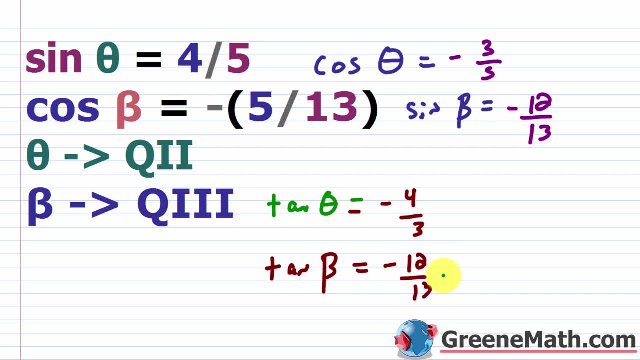 negative 12-thirteenths. Let me change my ink here And then times over here I'm going to flip this. So I'm going to do negative 13-fifths, And again stuff's going to cancel. So this cancels with this. 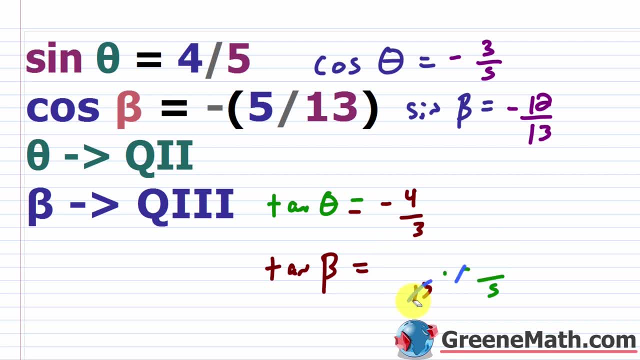 Negative cancels with negative, That's positive. So you have 12-fifths, right? So this is positive 12-fifths, Okay. So let me drag this back up. So let's cut this away and let's paste this in here. 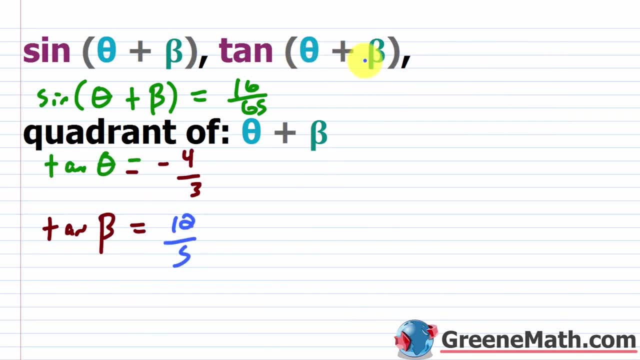 Okay, And let's see if we can figure out what the tangent of theta plus beta is. Again, I take the tangent of the first guy. Let me write this off to the side. So the tangent of theta plus beta: Okay, So the tangent of the first guy, which is negative four-thirds. 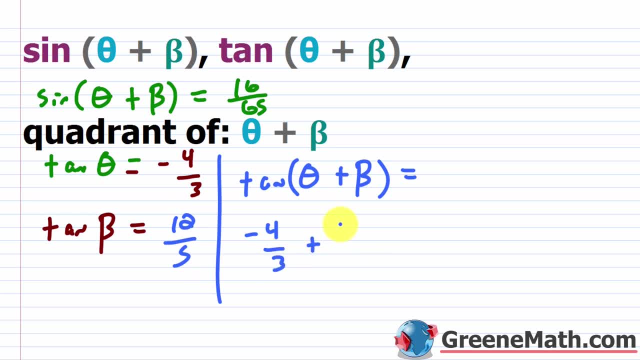 then plus the tangent of the second guy, which is 12-fifths. This is over. We want one Again. this is plus because it's the same as this. This is going to be minus, right? So this is always different, This is always the same. So one minus, multiply the two together. 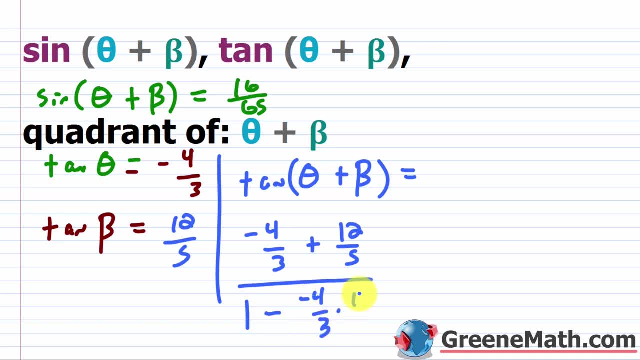 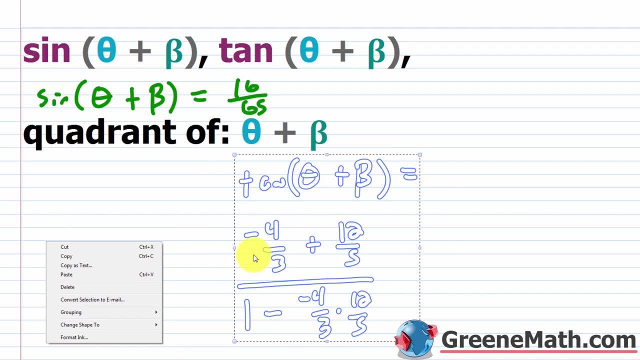 So it's negative. four-thirds times your 12-fifths. Okay, And let me get rid of this now. We don't need it, just so we have some room. So let's move this over. Let's move this over. Okay, Put this. 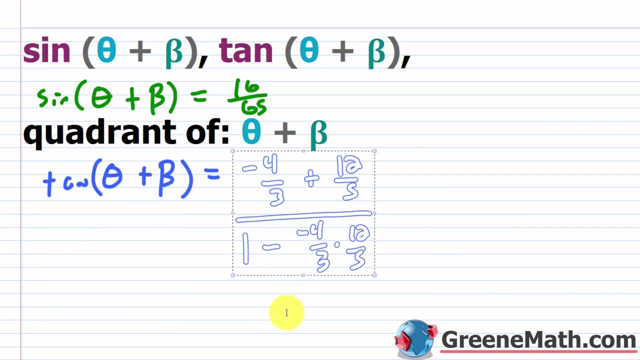 over here And I'm going to drag this up here a little bit And I'm just going to scroll down a little bit. We'll come back up in a second. So the best way to do this, let me just put equals over. 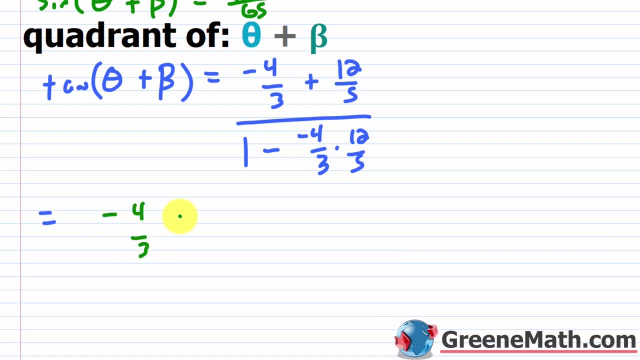 here. I'm not going to get a common denominator yet, So I'm going to go negative four-thirds plus 12-fifths over For this one. I'm just going to multiply: Negative four times 12 is going to be negative 48.. This is over. Three times five is 15.. And 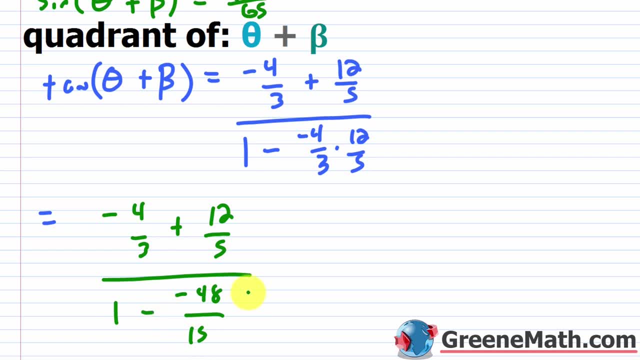 you've got one minus this, Okay. So what is the LCD? if I think about all the fractions involved, If I think about three- and that's a terrible three, so let me make that better. So if I think about this three here, let me get off the marker mode. So this guy, the three, the five and the. 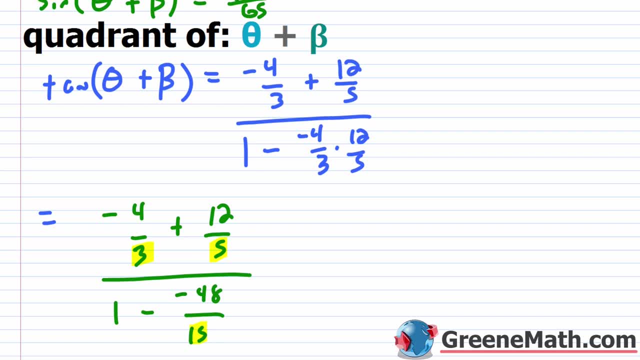 15.. Well, it's 15, right? So the quickest way to do this, in my opinion, is to multiply the top and bottom by 15.. Okay, So I'll save you a lot of time. I'm going to go ahead and do that. I'm going. 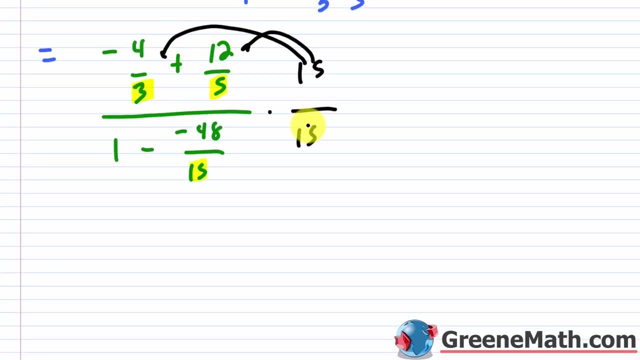 to save you a lot of time, We'll go ahead and distribute this here and here and then here and here. Okay, So, first off, minus a negative is the same as plus a positive. Okay, You can just change that right away. So you have to deal with it And you'd have: 15 divided by three is five, Five times. 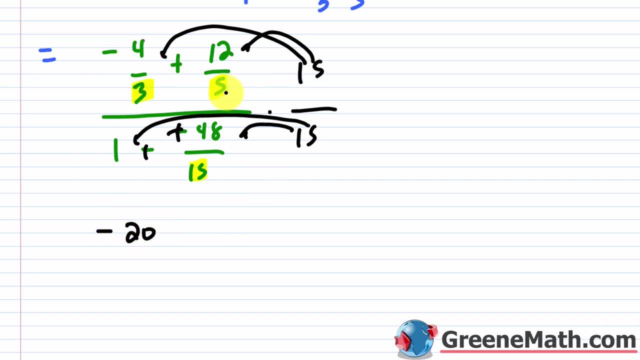 negative four is going to be negative 20.. Then 15 divided by five is three. Three times 12 is going to be 36.. So plus 36.. You can go ahead and do that if you want. You know that's going to be 16.. So 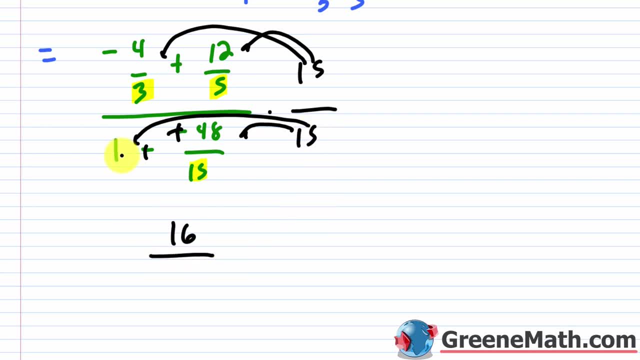 this is 16.. This is over. If you multiply 15 by one, that's 15.. And then 15 divided by 15 is one, So you just have plus 48 there. So what's 15 plus 48?? 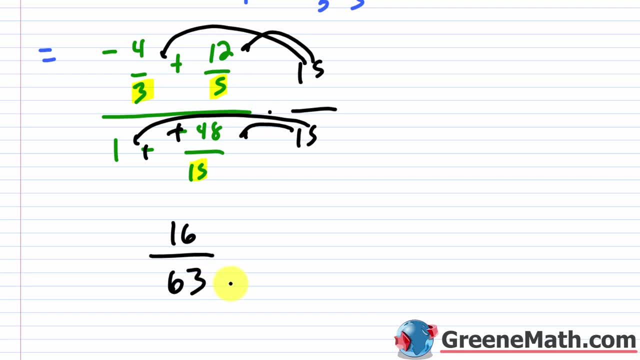 It's going to be 63. Okay, So this guy's going to be 16 over 63. And I could put equals there. But really I'm just going to erase all of this And I'll just put a little line here. 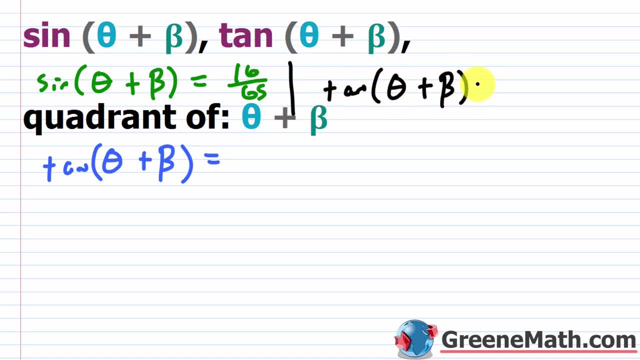 put, the tangent of theta plus beta is equal to- and let me just paste that in my 16 over 63.. Okay, So sine of theta plus beta is 16 over 65.. Tangent of theta plus beta is 16 over 63.. Now we want to think about, and I can just get rid of this: 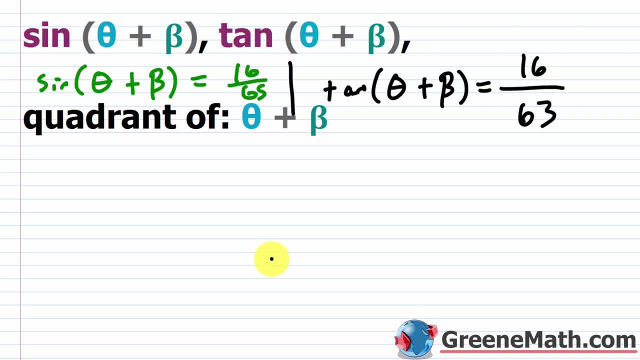 We want to think about the quadrant of theta plus beta. Well, I just want you to think about the sine. The sine of theta plus beta is positive, right? So sine is positive, Okay. The tangent of theta plus beta is also positive. So the tangent is also positive, Okay. So where is? 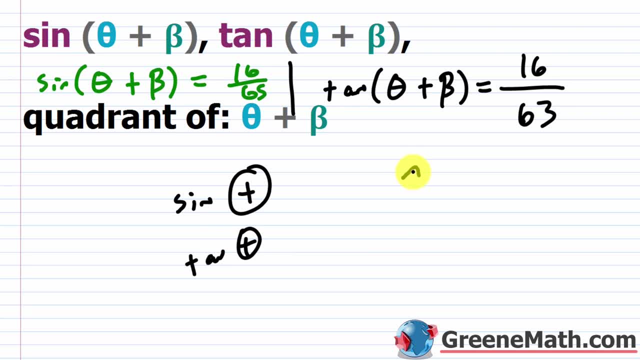 sine positive and also tangent positive. Remember, you can always draw your little coordinate plane And I know this is a terrible freehand draw, but it's all. students take calculus right? All you have your sine, your tangent and your cosine. Okay, So if we think, 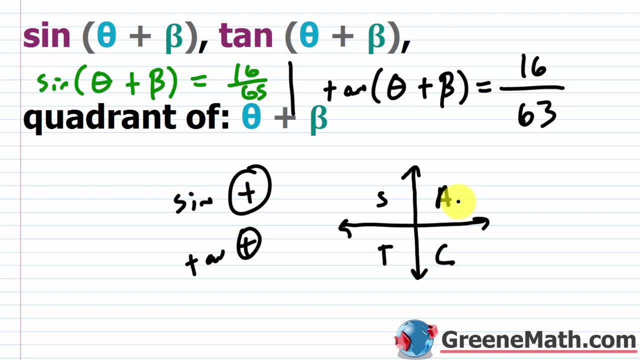 about sine: it's positive in quadrants one and two, and tangent is positive in quadrants one and three. So the only guy that meets both criteria here it's going to be quadrant one, Okay. So the quadrant of theta plus beta- okay, is going to be one. So this is going to be, we'll say, is: 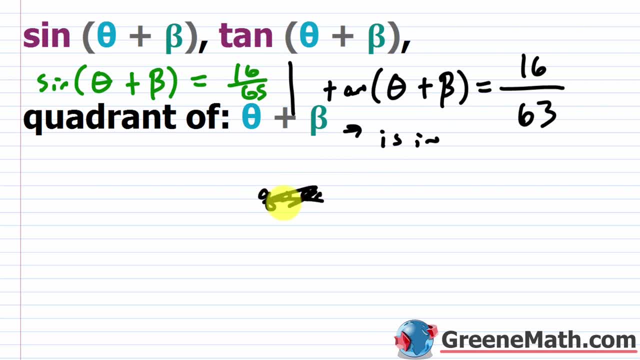 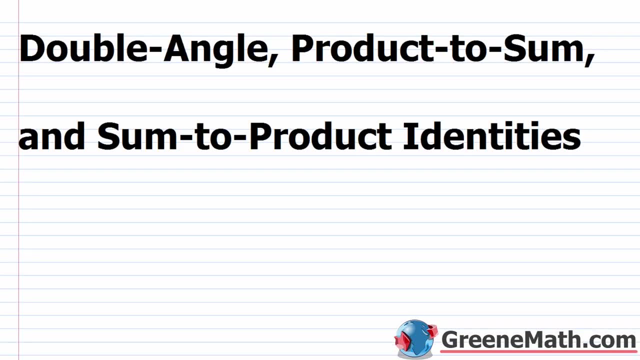 in quadrant, quadrant. I just probably put a capital Q, So quadrant one. In this lesson we want to talk about the double angle: the product, the sum, and also the sum to product identities. All right, So at this point, 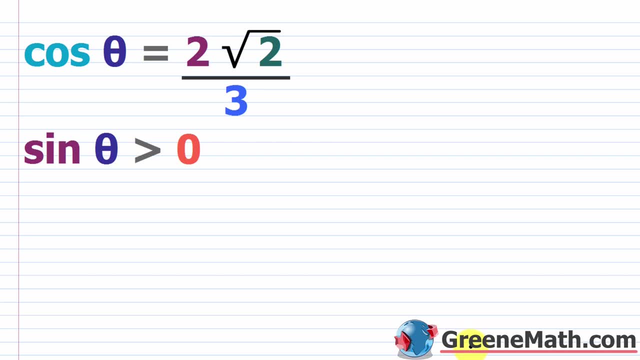 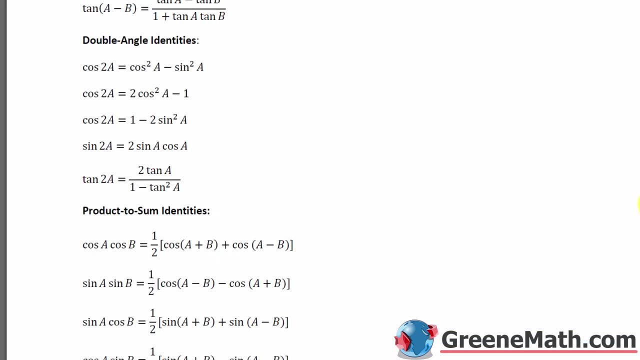 we've learned quite a few of the trigonometric identities. We just keep adding on to the ones that we already know. I'm just going to pop open this little worksheet here real quick. So this is the whole worksheet. If you go back up to the top, this is all the stuff we've already. 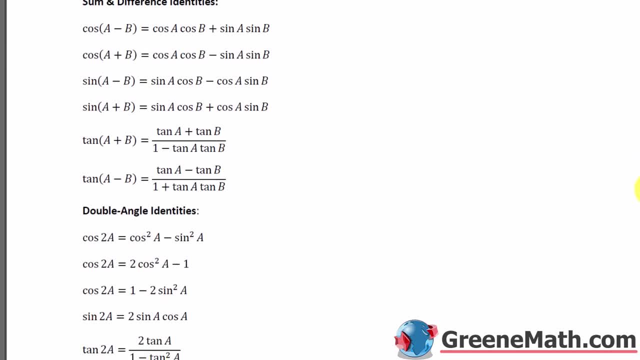 learned. So all of these guys we've already talked about and now we're getting into the double angle identities, And then again we've learned. you know we're going to work with this and we'll talk about the product to sum and the sum to product at the end of the video. 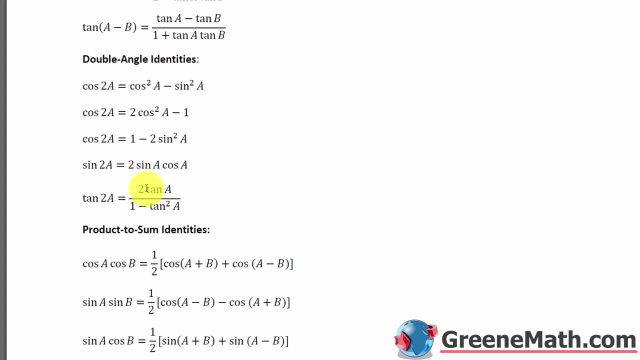 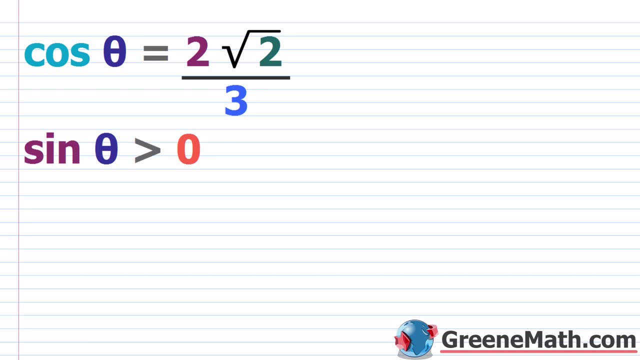 Right now we're going to focus on these, So you can either pause the video and write these down really quickly, or you can use the worksheet that's been provided. Okay, so the problem we're going to look at here is just going to be asking to find some trigonometric function values. 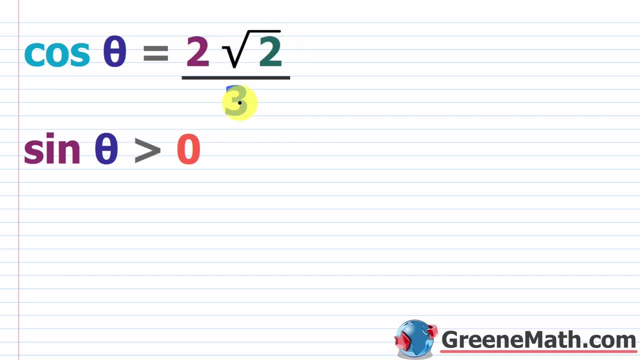 We have the cosine of theta is equal to two times square root of two over three, And we have that sine of theta is greater than zero, or you could just say positive, right? So basically, if it's cosine of theta is positive and sine of theta is positive, 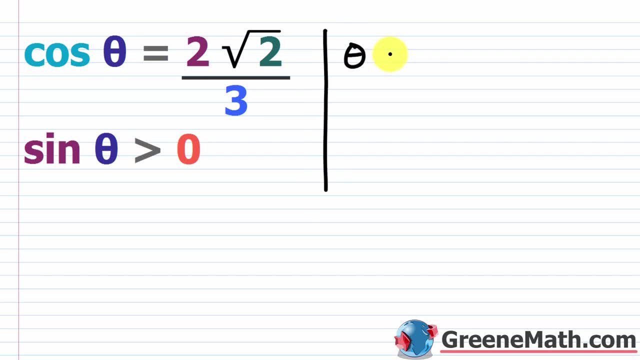 that tells me that we're in quadrant one, right? So we can say here that theta is in quadrant one, So we're going to need that piece of information. Now, what we're going to be asked to find is the cosine of two times theta, So we want to find the. 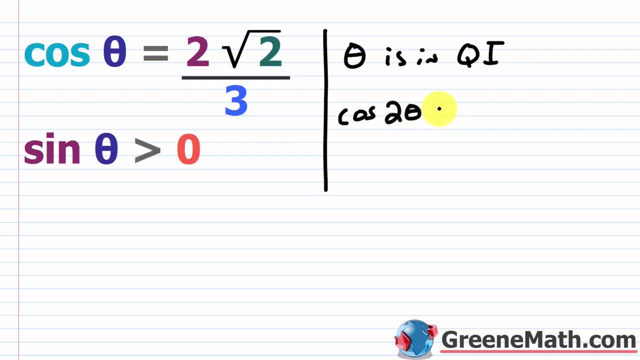 cosine of two times theta. We also want to find the sine of two times theta, Okay, And then also we want to find the tangent of two times theta. And of course, once you have these, you can use your reciprocal identities to find the other ones. I'm just going to do these three right here. 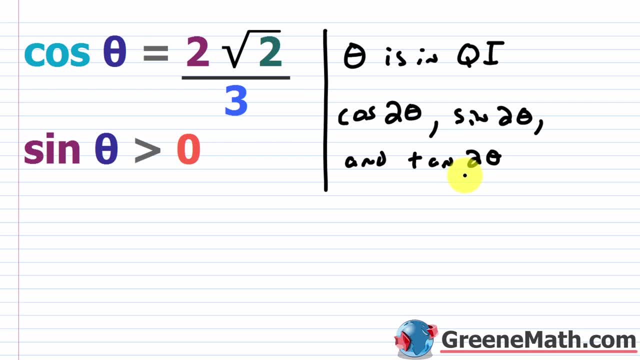 All right, So the first thing I'm going to do, what I'm going to focus on, is finding the sine of theta and the tangent of theta. Okay, And then we're going to use our identities to find the cosine of two times theta, the sine of two times theta and the tangent of two times theta. 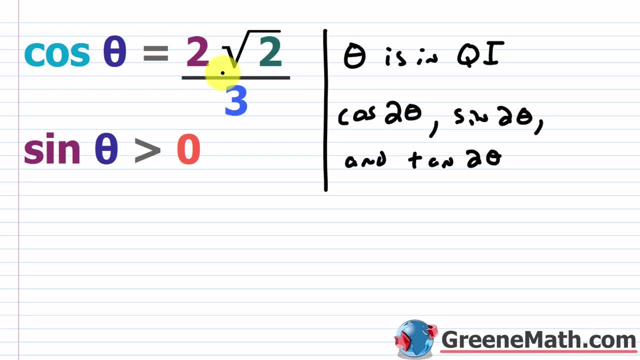 Okay. So if I'm given cosine of theta, how can I find sine of theta Again? we've done this a million times. One way we can do this: we can say that cosine squared, theta plus our sine squared is equal to one. Okay So, our Pythagorean identity, something we're really used to working with at this. 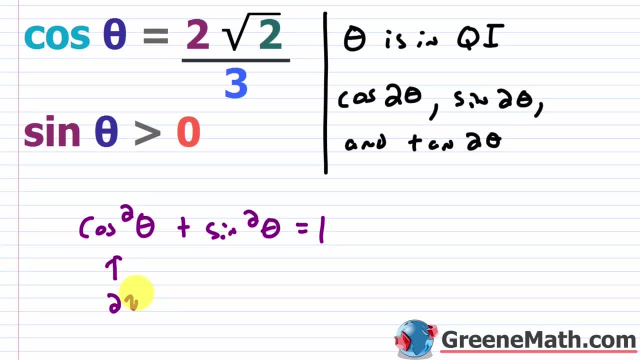 point. So for this guy, I'm going to plug in this two times square root of two over three and I'm just going to square this guy. Okay, Let me just copy this and go to a fresh sheet because we're going to run out of room here, So let's come down here and just paste this in, so we have lots of. 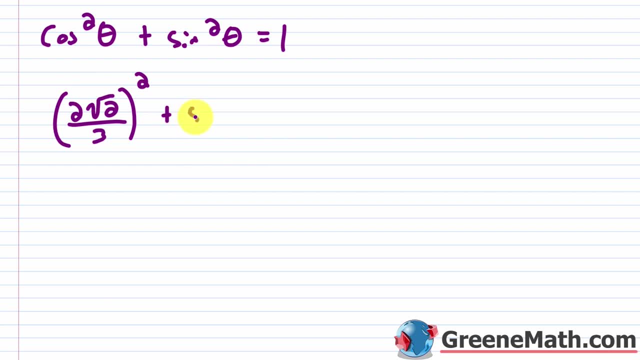 room. And then I'm just going to say, plus my sine, squared theta is equal to one, Okay. So from here, if I squared two, I would get four. If I squared the square root of two, that's two, Okay. And if I squared three, I would get nine. So basically, four times. 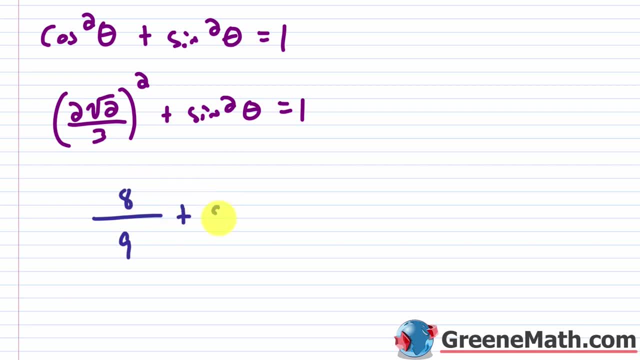 two is eight, So this is eight ninths. Then, plus your sine, squared theta is equal to one. I'm just kind of dragging this up here And from here I'm just going to say that I have sine squared theta is equal to. I'm going to subtract eight ninths away from each side of the equation. 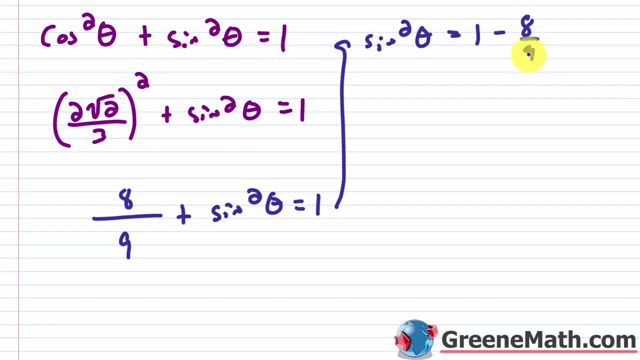 So I'm going to put one minus eight ninths. Okay, And again, all I did was subtract it from both sides of the equation, And so now what I have is minus eight ninths, So I'm going to put one minus my sine. squared theta is equal to if I write this as nine over nine, so I have a common 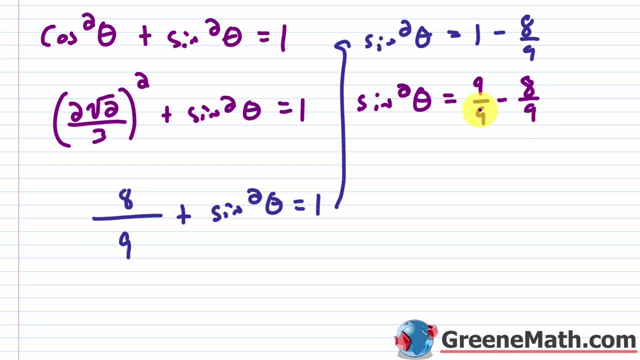 denominator, and then I'm subtracting away this eight ninths. here, this on the right-hand side is going to be one ninth. So I would say: sine squared, theta okay is equal to one ninth, Okay. Now, from here, in order to get rid of this kind of squaring operation, I'm going to take the square root of. 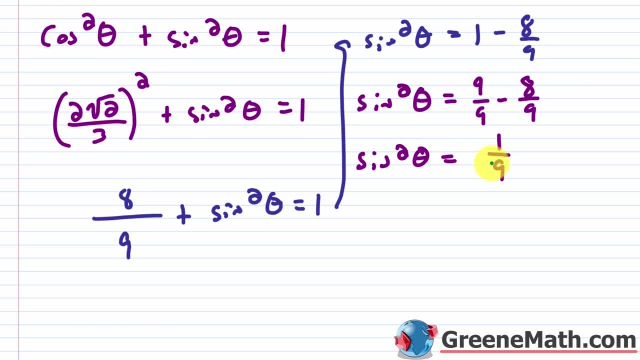 each side. Normally, again, you do the plus or minus on the right-hand side, but because we're, I know that sine is positive, so I want the principal square root. So I'm just going to say that the sine of theta here is going to be the principal square root. Let me show this fully. So 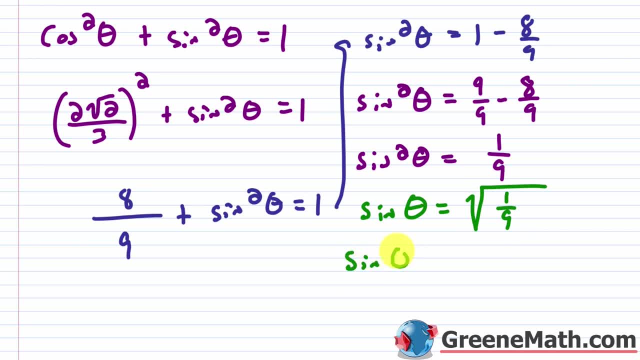 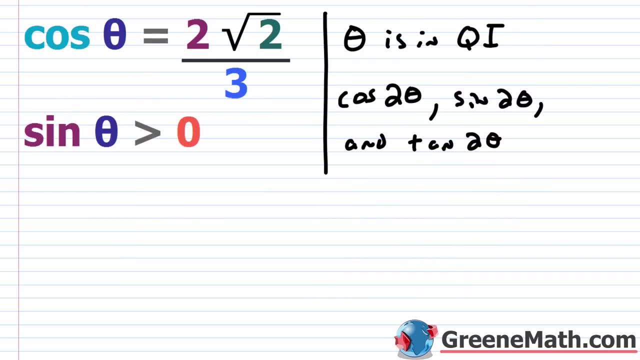 the principal square root of one, ninth. Okay, So the sine of theta is equal to square root of one is one. square root of nine is three. Okay, So let me just write this up here, that the sine of theta, so the sine of theta, is equal to one third. Okay, And we'll come back up and we'll use this. 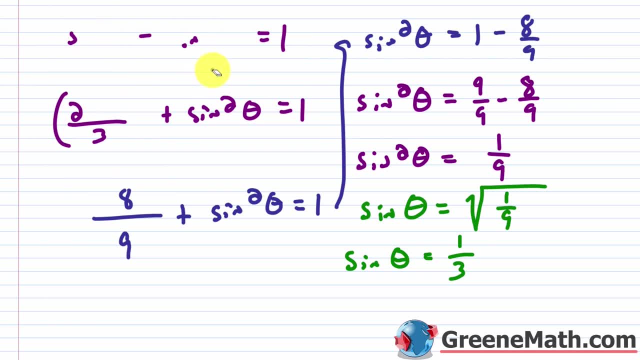 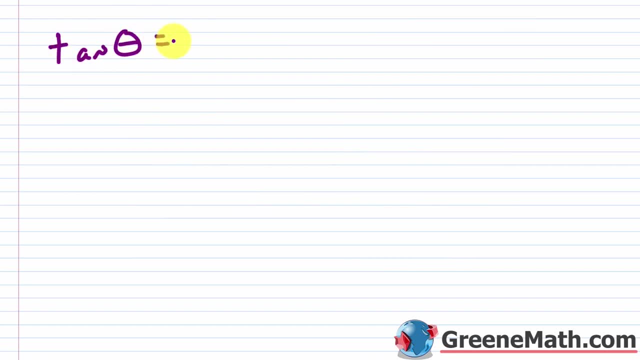 Let's come back down here for a second. Let me erase all of this. So I'm also going to need my tangent of theta. So the tangent of theta. we all know that this is the sine of theta divided by the cosine of theta. So the sine of theta we just found was one third. 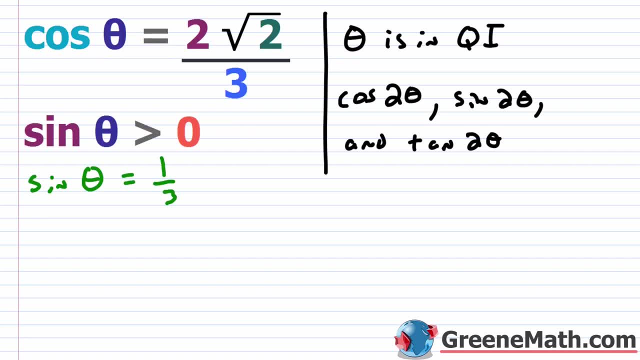 Okay, And the cosine of theta. if I go back up here, it's two times square root of two over three. Okay, But because I'm going to be dividing fractions, I'm going to go ahead and flip that guy and multiply. So this is three over two times square root of two. Okay, So what's going to happen? 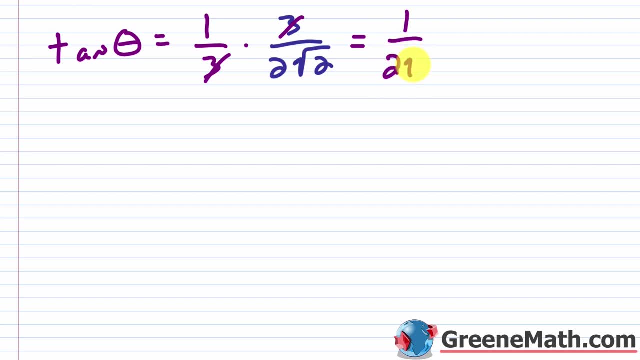 is, the threes are going to cancel And I have one over two times the square root of two. I want to rationalize the denominator here, So I'm going to multiply by the square root of two over the square root of two. Okay, So basically, if I think about what I'm going to have here in the numerator, 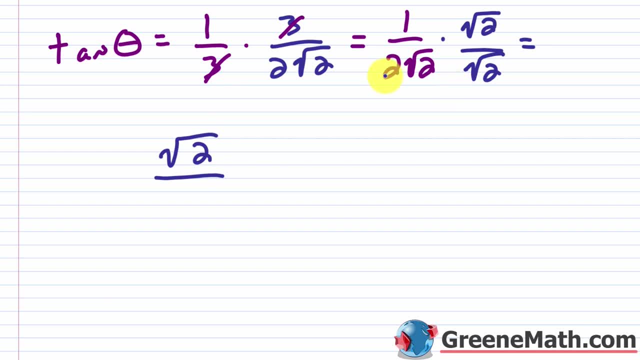 it's just the square root of two. In the denominator it's two times the square root of two, times the square root of two. Square root of two times square root of two is two. So two times two would be four. Okay, So the tangent of theta is the square root of two over four. So let's just. 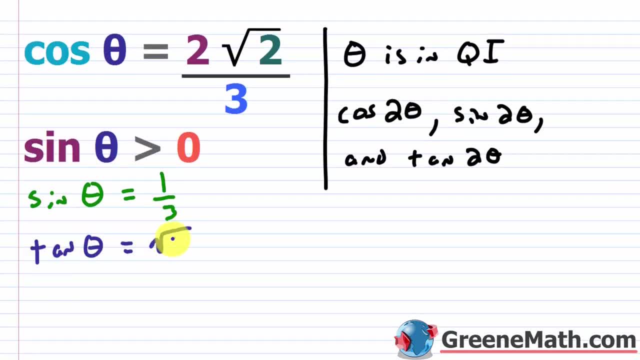 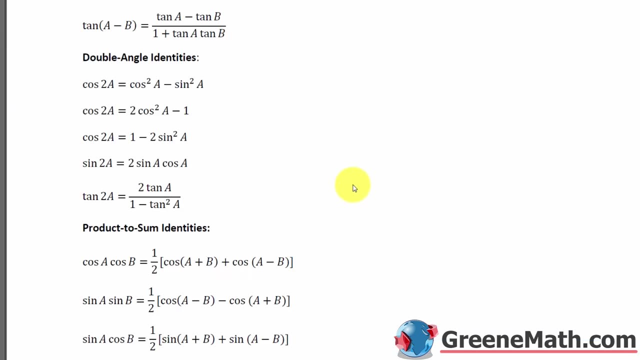 write this here, that the tangent of theta is the square root of two over four. Okay, So now let's go ahead and find the cosine of two times theta, the sine of two times theta and the tangent of two times theta. So for the cosine of two times theta let's go back to our little sheet here. So we have. 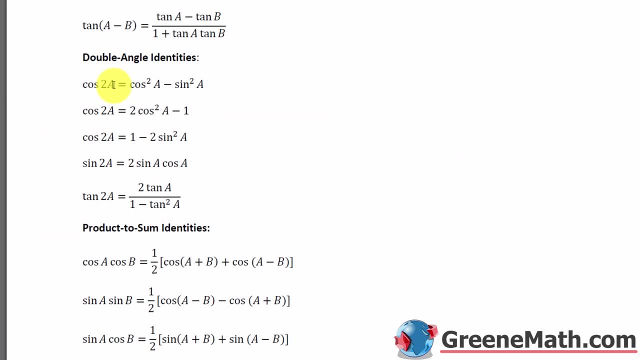 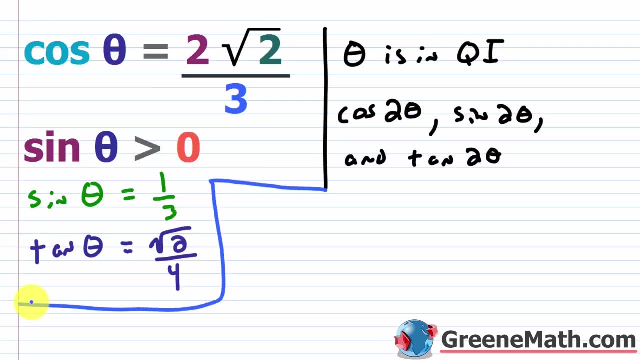 cosine of 2a. You could plug in theta for a or x or whatever you want to do. It's cosine squared of a minus sine squared of a, So that's pretty easy to do. So let's make a little border here And 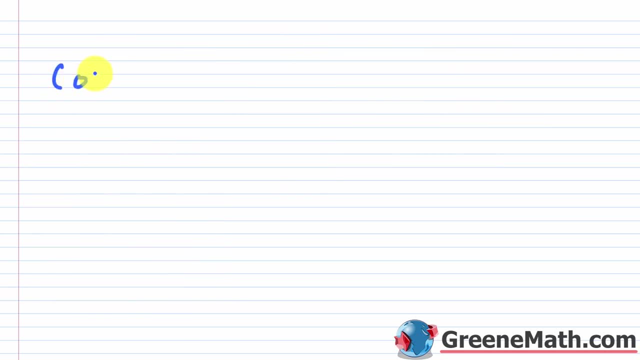 actually I'll probably be better off just going to the other sheet. So we'll say: cosine of two times theta is going to be equal to cosine squared theta minus sine squared theta. Okay, So I'm just going to plug in: So cosine of two times theta is equal. to remember, our cosine of theta was two times the. 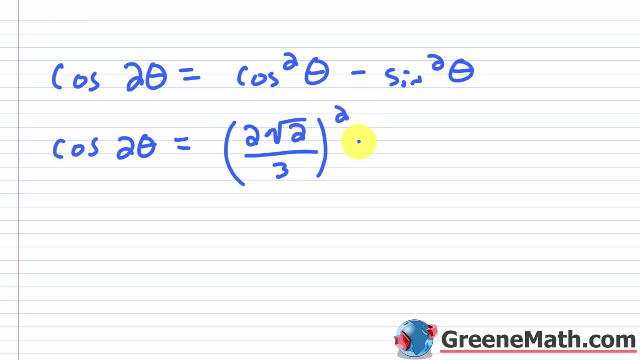 square root of two over three. Hey, this guy's going to be squared. Then minus, remember our sine squared theta. you might remember this was one ninth, but basically sine of theta was one third, right? So I'm going to put one third here and square it, and that's going to give me one. 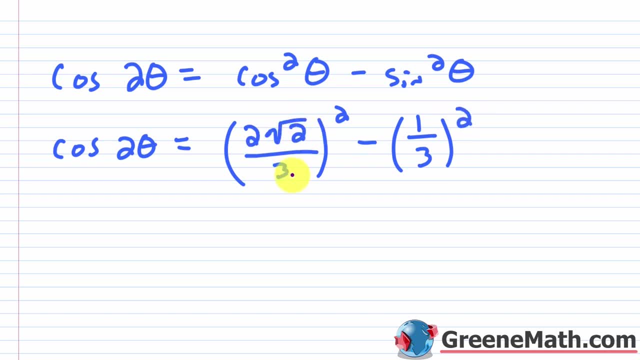 ninth, Okay. So if you remember from earlier, when we squared this, we got eight ninths right, Because two squared is four, square root of two squared is two. four times two is eight, Okay, And basically three squared is nine. So this is eight ninths minus. let me put equals over here. I'll just 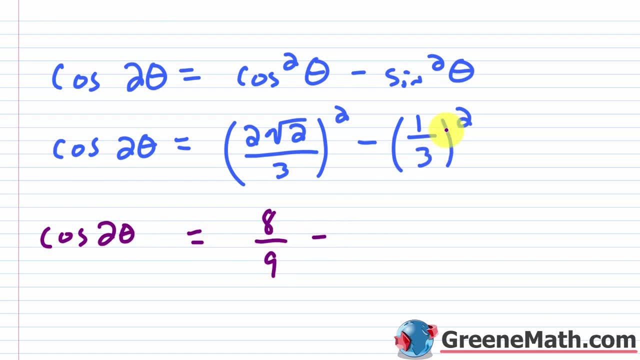 write the whole thing out. So cosine of two theta is equal to eight ninths minus again, if you square this, you get one ninth. Okay. So this gives me a final result here of seven ninths. So this is my sine of two theta, Okay. So let's come up here and put that our cosine of two theta is equal to: 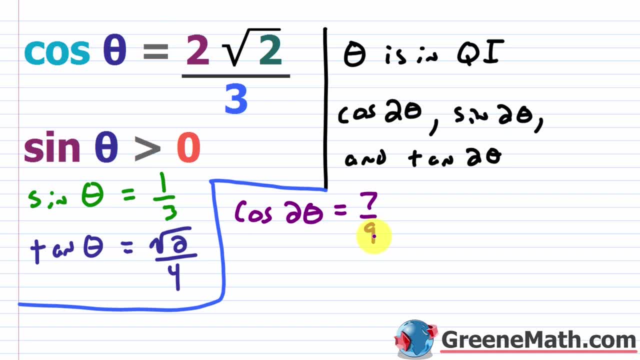 seven, ninths. Now, if you're asked for the secant of theta, you would just flip that and get nine, sevenths. Okay, But we're not asked for that here. So then now I want to find the sine of two theta. 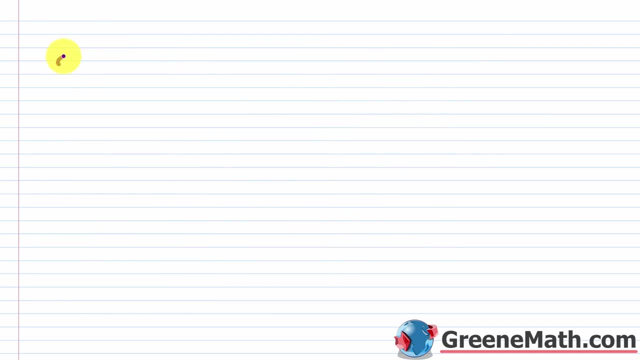 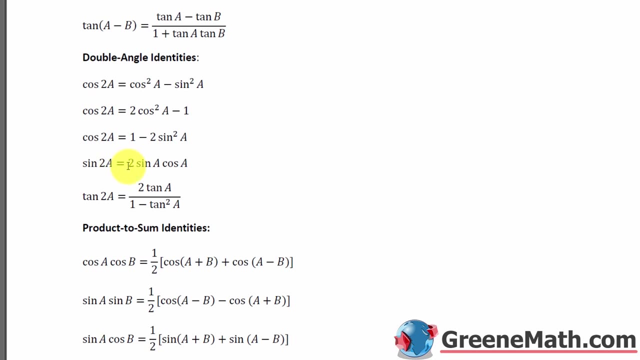 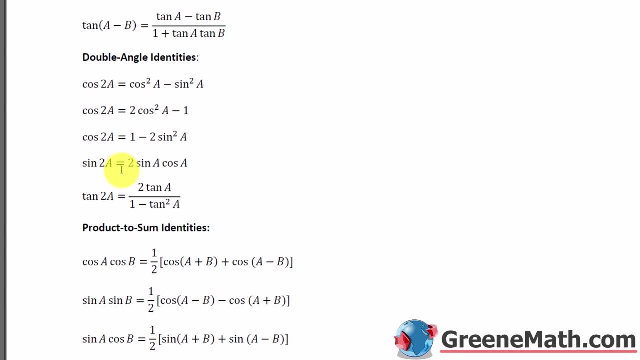 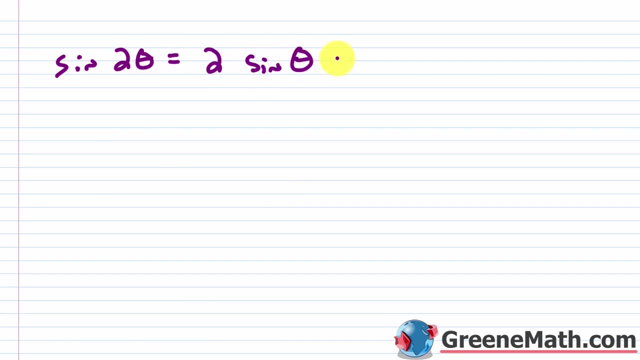 again, you can just plug in. you can say: the sine of two times theta is equal to two times the sine of theta times the cosine of theta. So this is equal to two times the sine of theta times the cosine of theta. Well, again, we know the sine of theta is one third. So this is one third And we 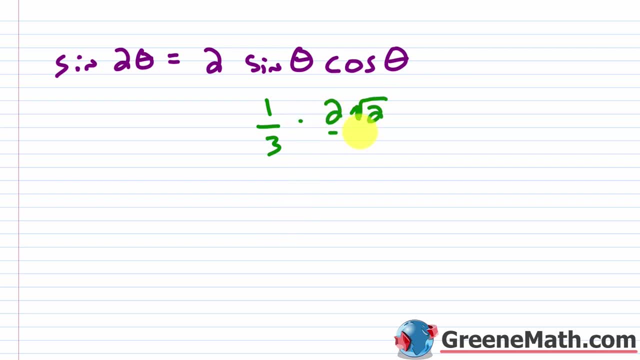 know, the cosine of theta is two times the square root of two over three. So let me put my two in here And let me put sine of two theta like this. So let me write this again over here: Let me put sine of two times theta And let me put sine of two theta, And let me put sine of two theta, And. 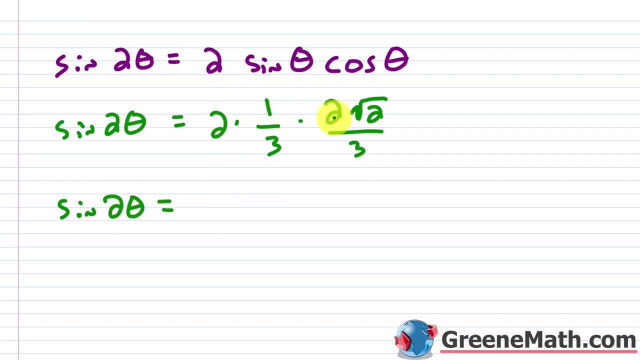 let me put: sine of two theta is equal to. basically, I'm just going to multiply across two times one times two is going to be four. then times the square root of two over three times three is nine. Okay, so sine of two theta is equal to four times square root of two over nine. So 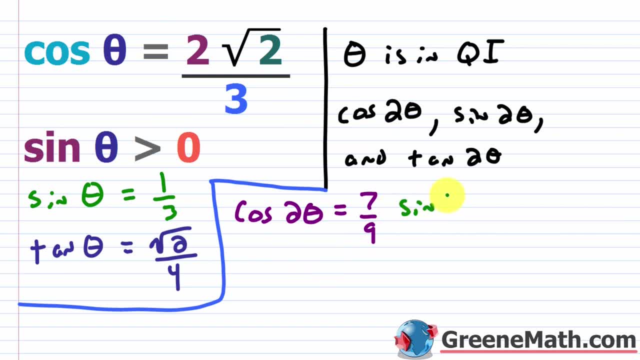 let me just move this down a little bit, Or actually I can put it over here. So the sine of two times theta is equal to four times the square root of two over our nine. And again you could flip this to find the cosecant of two theta. Okay, But again you'd have to rationalize. 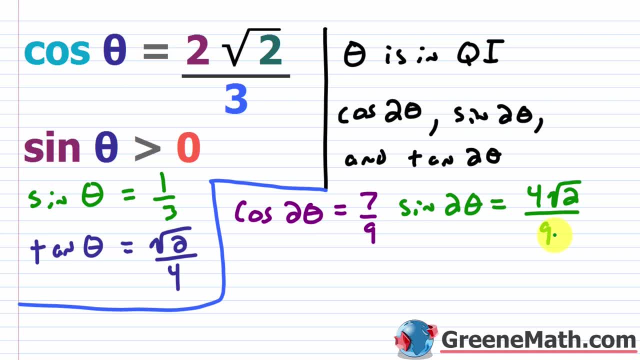 the denominator there. We're not asked for that, So we're going to put sine of two times theta here, So we're not going to do that, Okay. so, lastly, we want the tangent, the tangent of two theta. So how do we find this? Well, essentially, all I need to do is take this guy right here and 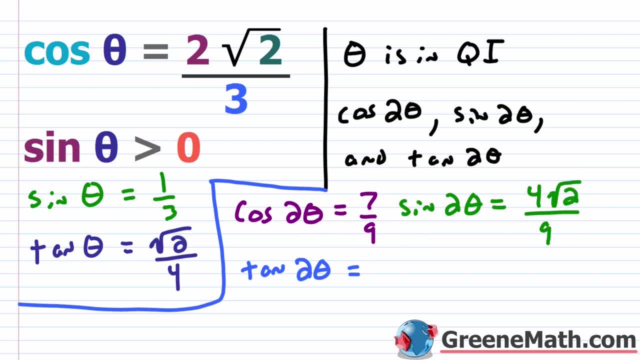 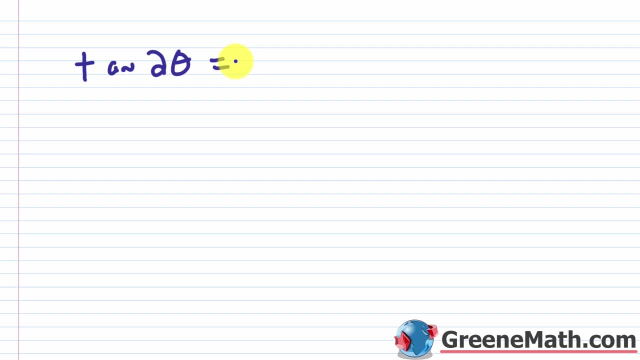 divide it by this guy right here, Or I can use my formula. So let's see this both ways. So for the tangent of two times theta- the first way we're going to do it, probably the easier way- you basically take your sine of two times theta, which again is four times square root of two over nine. 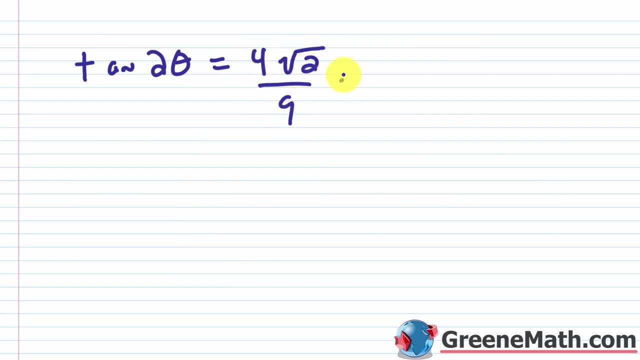 So four times square root of two over nine. we're going to multiply it by the reciprocal of this cosine of two theta, which is seven, ninths. So if you flip that you get nine, sevenths Again. I'm flipping that because if you're dividing, 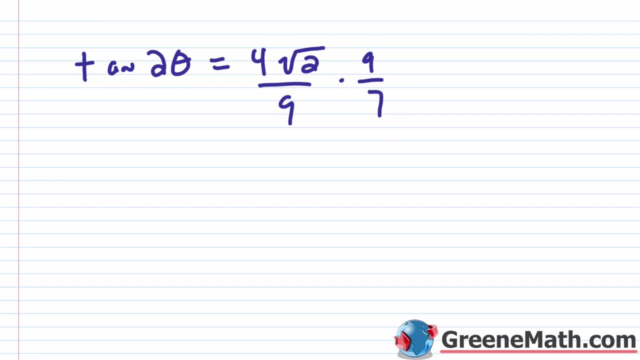 fractions. you take the first fraction multiply by the reciprocal of the second. So this is going to cancel. we're gonna be left with four times square root of two over seven. So that's the quickest way, That's the way you probably want to do this, So let's come back up here. So four times. 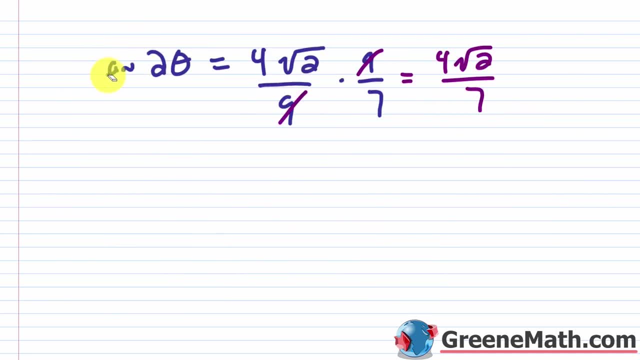 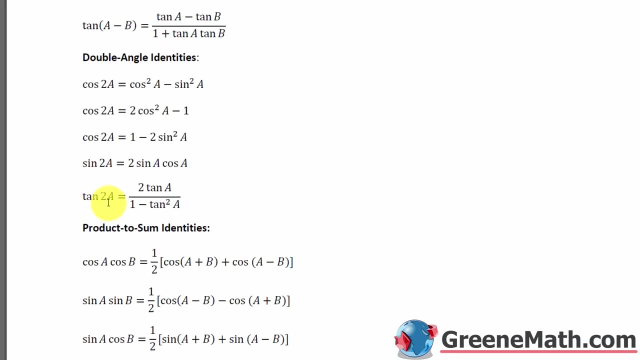 square root of two over seven. Now the other way, and I just want to show you this with the identities. it's a little bit longer, but I think you should see it. Let's pop this open. We have the tangent of two. a is equal to. 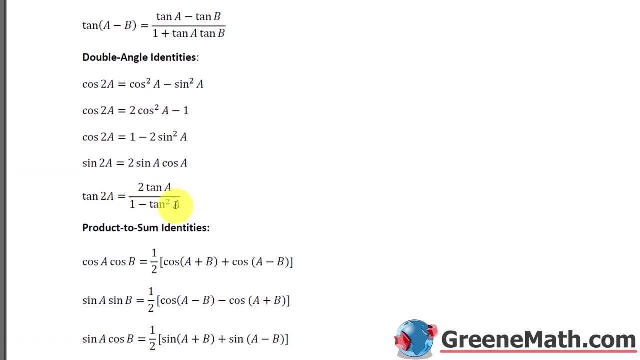 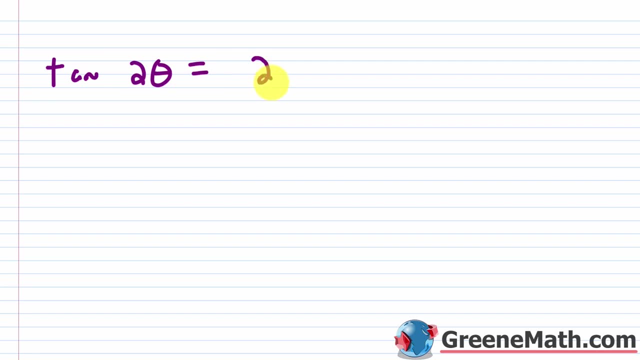 two times the tangent of a over one minus tangent squared of a. Okay, so let's come down here and say that the tangent of two times theta is equal to two times the tangent of theta over one minus tangent tangent squared theta. Okay, so what is the tangent of theta if we go back up? 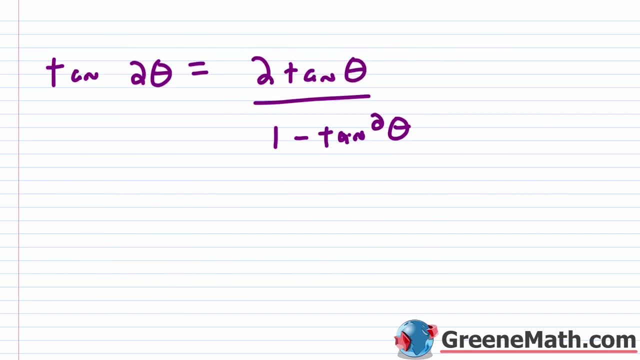 the tangent of theta was square root of two over four. so let's come back over here and I'm just going to put this over here. So the tangent of theta was a square root of two over four. So we would start with, and let me 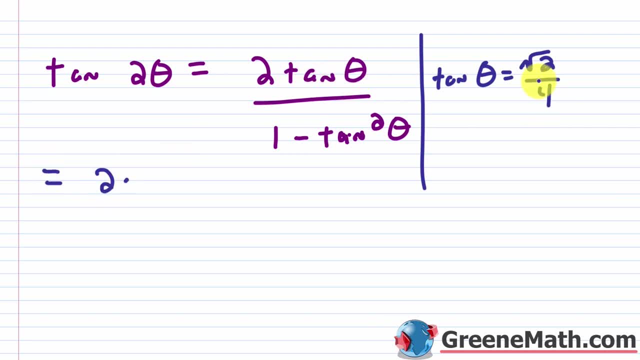 just put equals over here, two times this guy right here, which is square root of two over four, okay over one, minus tangent squared theta. so I'm just gonna square this guy. So if I square, let me just show this so that: so if I square the square root of two, 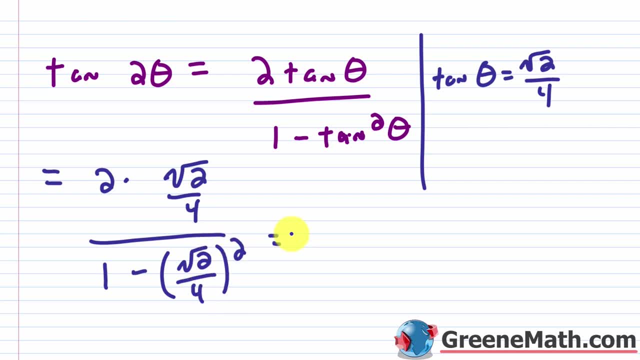 I'm going to get two. If I square for, I get 16.. Okay, so I'm gonna go ahead and say this is multiply across. i'll say this is 2 times square root of 2 over 4 over, you would have 1 minus. 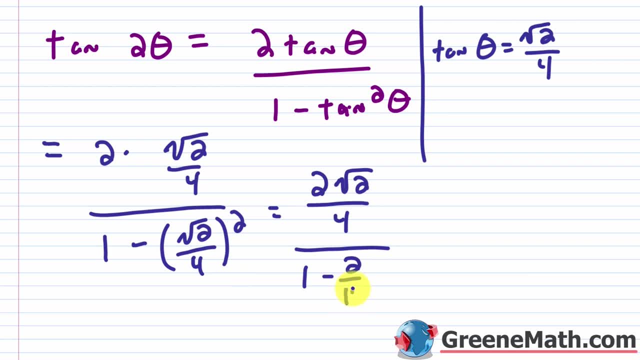 again, if i square square root of 2, i get 2. if i square 4, i get 16. okay, let me scroll down and get a little bit of room going here so we can see what's going on. it's probably quicker for me to. 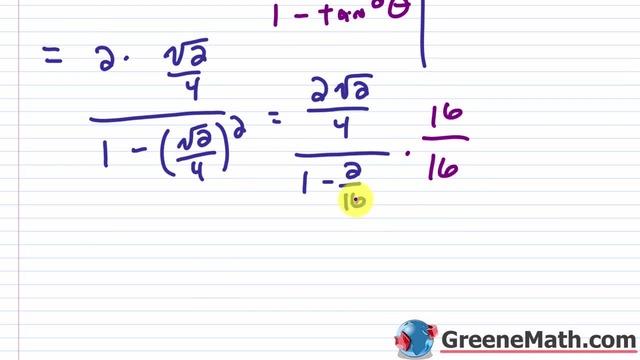 just multiply this by 16 over 16, that will cancel all my denominators. so 16 times this guy the 16 would cancel with the 4 and give me a 4. so you'd have 4 times 2, which is 8. so let me put 8 times. 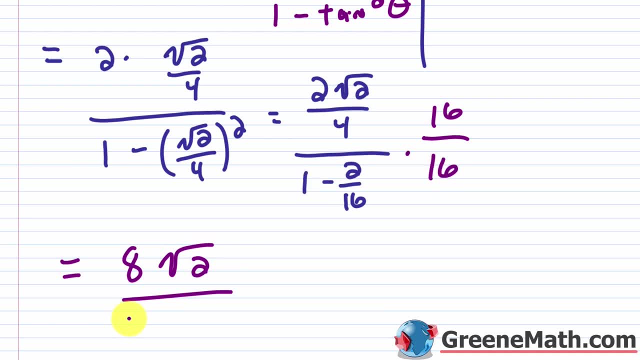 the square root of 2 here and then down here 16 times. 1 is 16 and then minus 16 times this guy right here the 16s would cancel. so i just have 2, okay, so that's probably a quicker way versus what. 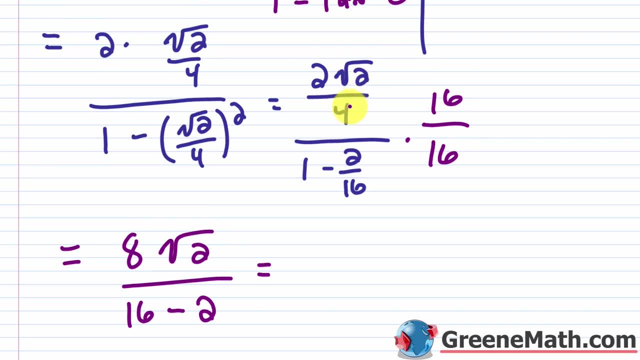 i was going to do, which is basically to work with these guys individually. okay, so now 16 minus 2 is going to be 14. so this is 8 times square root of 2 over 14. okay, and basically i can cancel this 8 and this 14. they're each divisible by 2, so this is going to be 4 and this is going to be. 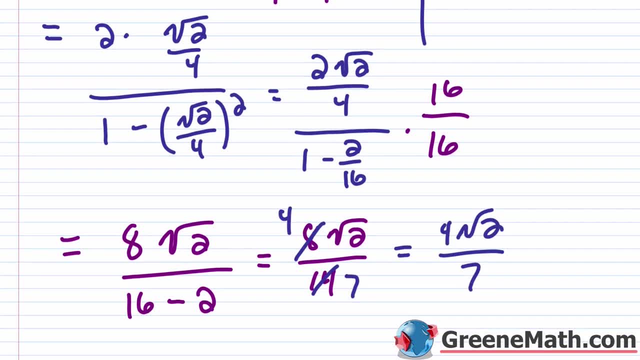 16.. right, so we get 4 times square root of 2 over 7 and you see that's what we got before, right? so it's much quicker if you have the sine of 2 times theta and the cosine of 2 times theta to just work. 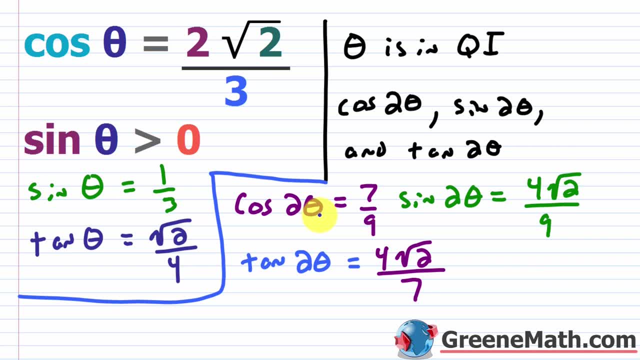 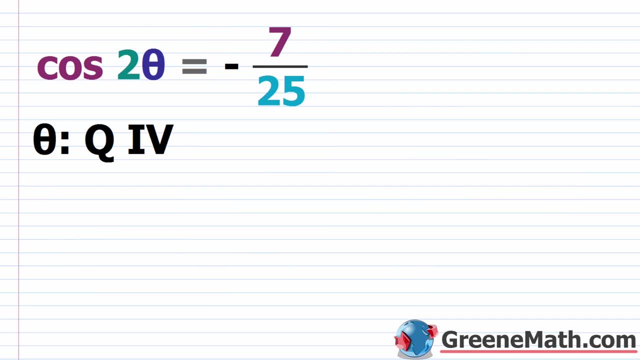 with that versus using the formula. but sometimes you're told to show it on a test or something like that. so if you do it the alternative way, using the double angle identity, it works the same, all right. so now we're going to look at a similar problem, but it's going to go in reverse. so now, 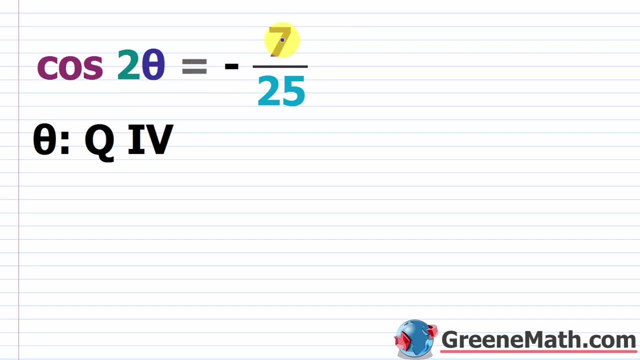 we're given the cosine of 2 times theta. in this case it's equal to the negative of 7 over 25. we're told that the cosine of 2 times theta is equal to the negative of 7 over 25, and we're told: 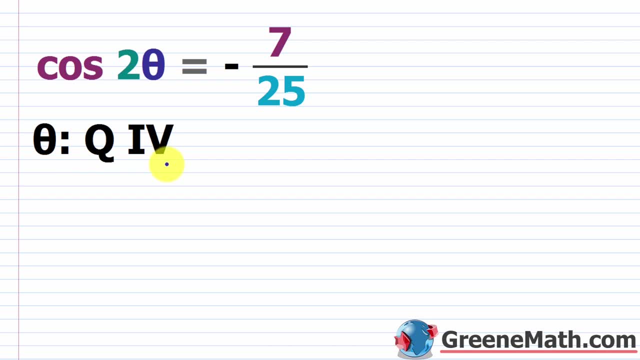 that the cosine of theta is in quadrant four. now you might be thinking that the cosine of theta should be positive in quadrant four, but remember, this is the cosine of 2 times theta. okay, so not the cosine of theta, this is cosine of 2 times theta. so what we're going to find here is the. 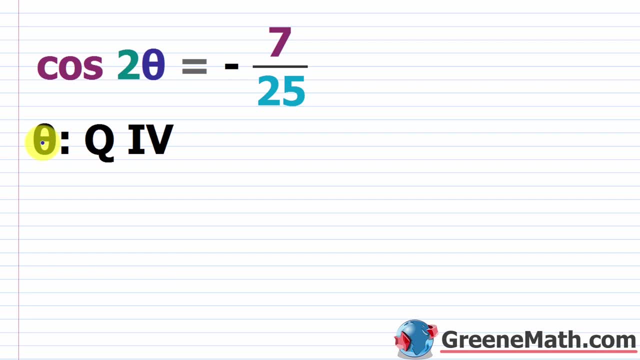 six trigonometric functions, those values for theta. okay, so basically i would start off by finding my sine of theta. i can then use that to find the cosine of theta and from those two guys i can basically find all the rest. right, really easy to do. so how am i going to find the sine of? 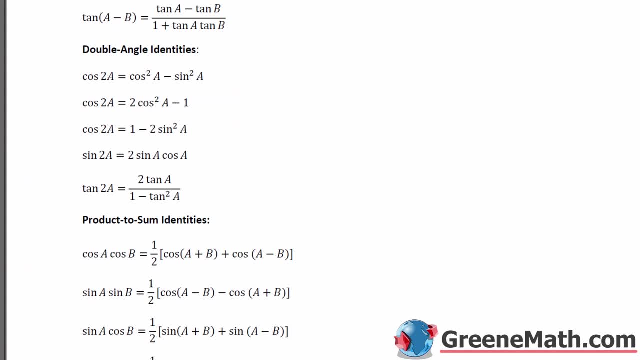 given this information, Let's go back to our little worksheet, or you could say handout, And basically, if you look here, you have this guy right here which would work pretty nicely. you have, the cosine of 2a is equal to one minus two times sine squared of a, So let's use that. 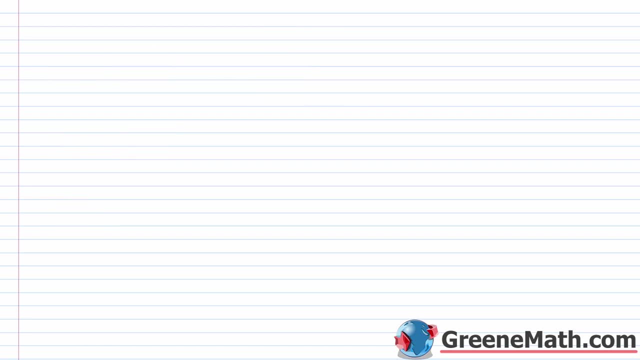 So we have the cosine. let me just on another sheet. So we have the cosine of two times. in this case I think it was theta. so it was theta is going to be equal to one minus two times sine squared theta. Okay, now I know what cosine of two times theta is. right, I'm given that, as 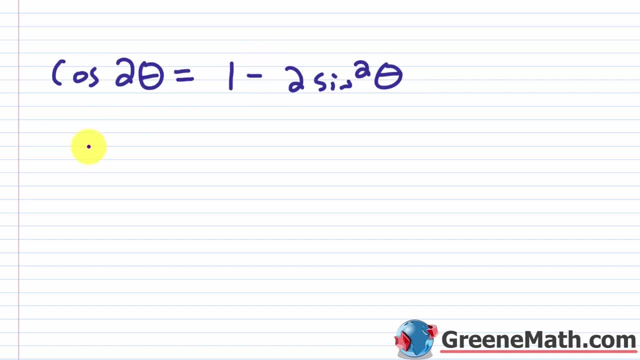 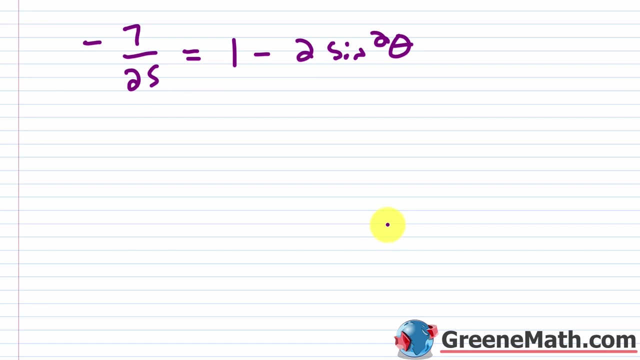 negative seven over 25.. So just plug in for that. So we're going to say this is negative seven over 25,. okay is equal to one minus two times sine squared theta. Alright. so from here let's go down a little bit, get some room going. I'm going to basically flip this around. 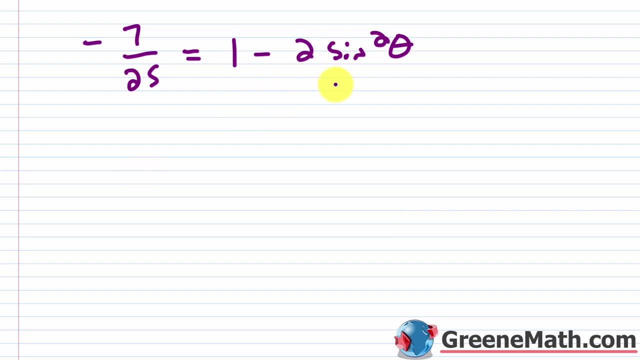 I want what I'm solving for on the left. So I'm going to add two times sine squared theta to both sides. So I'd have two times sine squared theta. okay is equal to- I'm going to leave this guy over here and I'm going to add seven, 25th to both sides. So basically I'm going to have 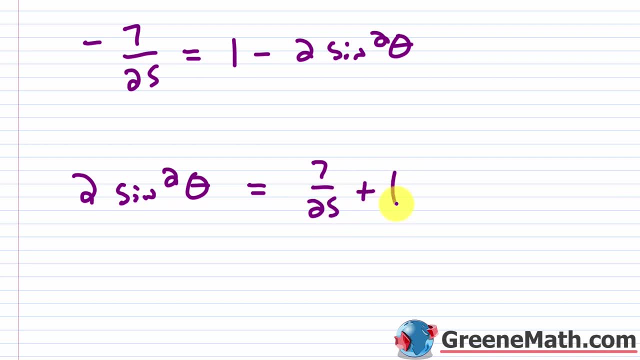 seven over 25, plus one over here. Okay, so all I did was just kind of swap things around, just adding and subtracting the same thing to both sides of an equation which is legal. Okay, so basically what I want to do at this point. 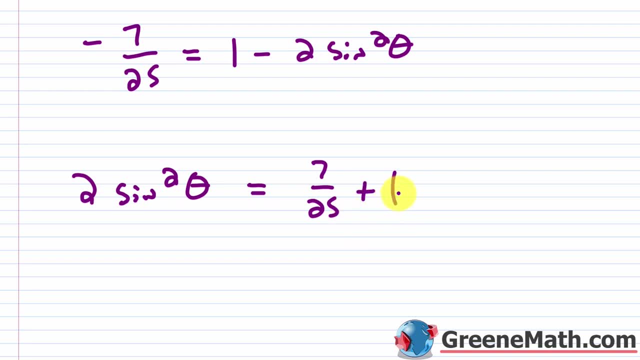 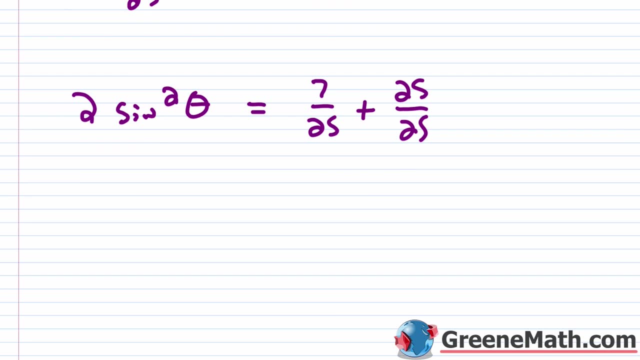 is go ahead and add seven, 25th plus one. So I'm just going to write this as 25 over 25.. And this would give me 32 over 25.. Okay, so I would have over here two times sine squared theta. 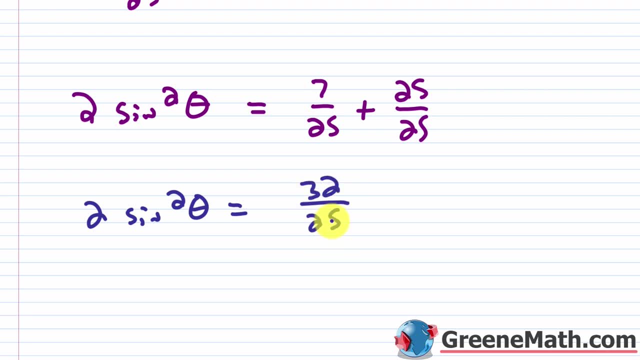 is equal to 32 over 25.. I have this two that I want to get rid of, So I can multiply both sides by a half. So let's multiply this side by a half and this side by a half And basically this is going to cancel out, And over here, this would cancel with this. 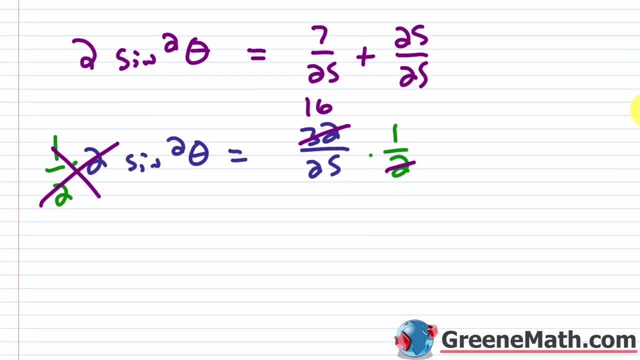 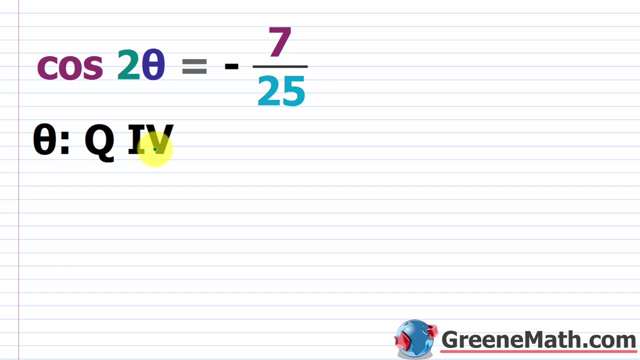 this is going to give me 16.. Okay, so now let me keep scrolling down here. we have that sine squared, theta is equal to. you have 16 over 25.. Okay, so you have to take the square root of each side again. if we go back up, we are told that theta is in quadrant four. we know that the sine 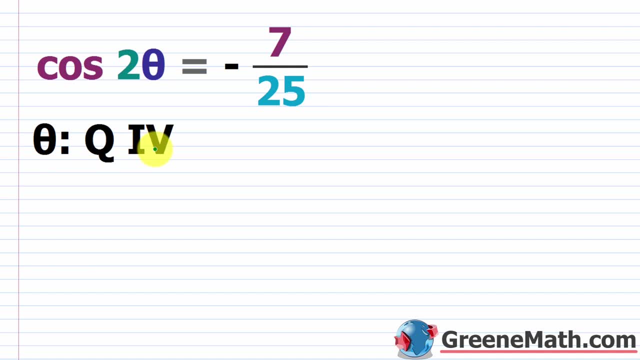 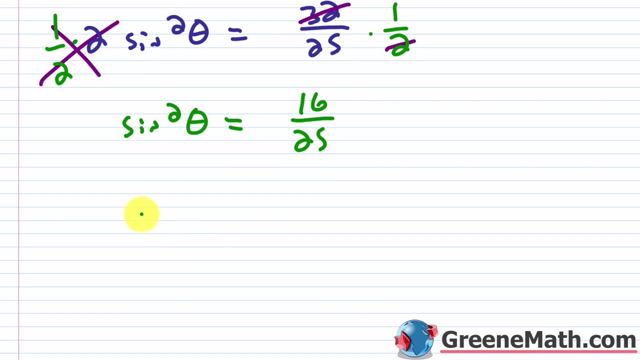 of theta, if it's in quadrant four is going to be negative right, Because sine is positive in quadrants one and two. So if we come back here, what I want to do is take the negative square root of this right hand side. 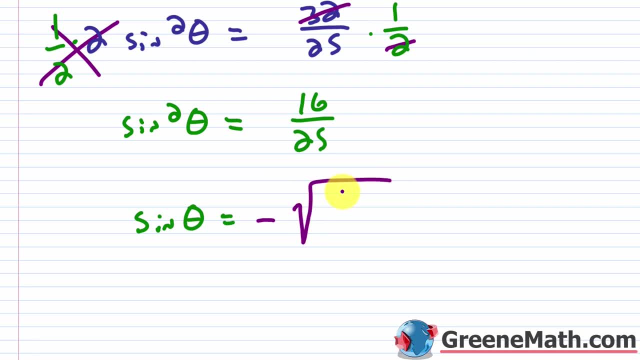 theta is equal to- I'll go- the negative of the square root of 16 over 25.. So the sine of theta is equal to the negative of square root of 16 is four. square root of 25 is five. So sine of theta. 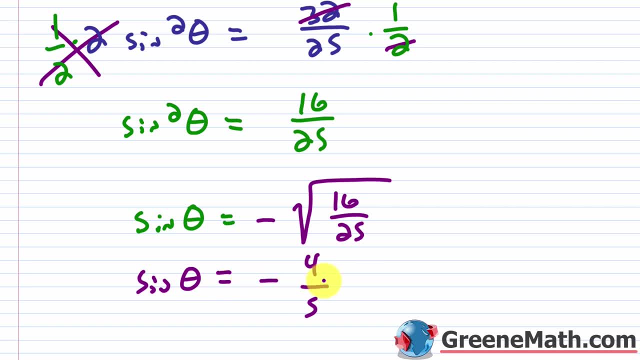 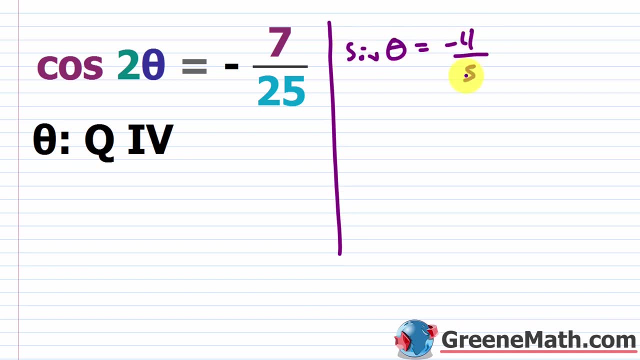 here is equal to the negative of four fifths. Okay, so let's go back up And let's put right here: the sine of theta is equal to negative four fifths. Alright, so how do we find the cosine of theta and all the rest of them? Well, basically, at this point we can just use: 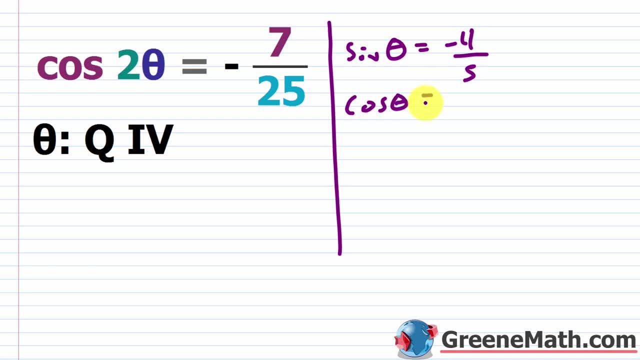 our regular identities that we've been working with. I can use the Pythagorean identity to get this guy. So we know that sine squared theta plus cosine squared theta equals one. So I'm gonna have my negative four fifths for my sine of theta. I'm going to square that plus my cosine squared theta. 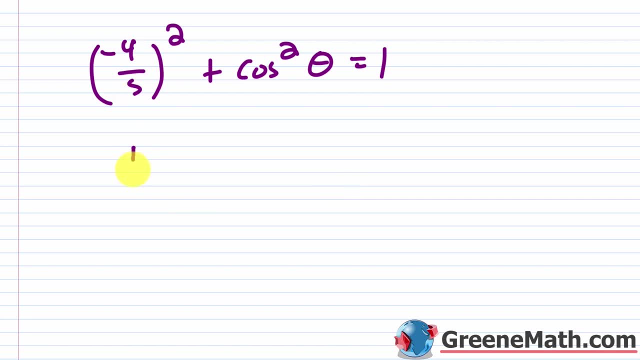 this equals one. okay, So if we square this, we get our 16 over 25.. Then, plus our cosine squared theta, this equals one. let's subtract this away from both sides, So I'm going to have: cosine squared theta is equal to. I'm just going to write this as 25.. 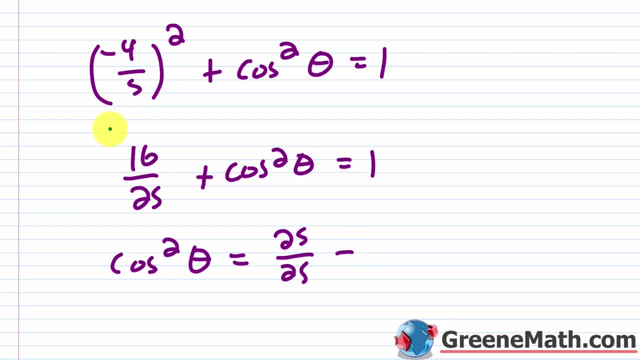 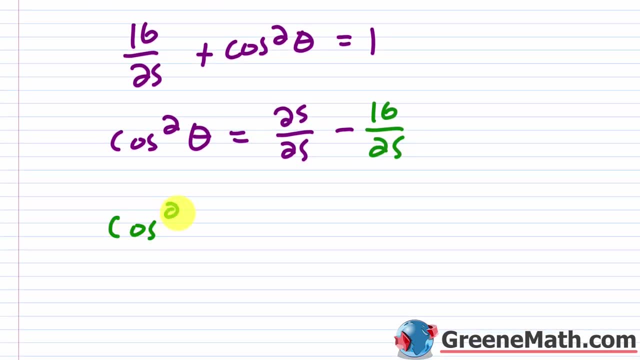 over 25. to speed this up- And over here I'm going to put minus again- I'm subtracting this away from each side, So 16 over 25.. Okay, so from here it's pretty easy. We have cosine squared. 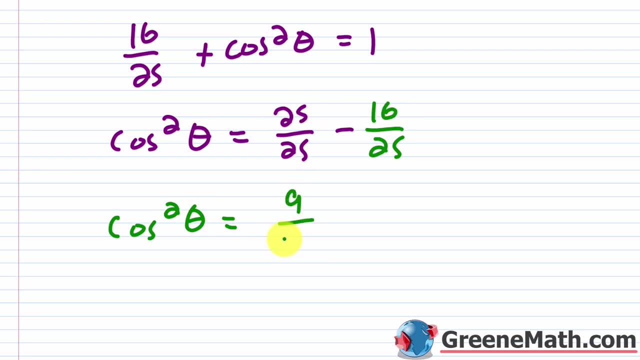 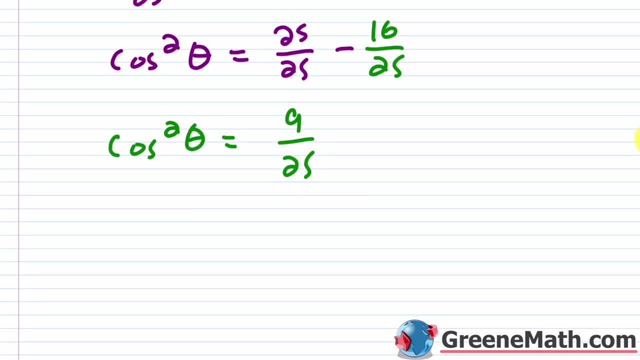 theta is equal to 25 minus 16 is nine, So this is nine over 25.. Okay, so we're in quadrant four. cosine is going to be positive in quadrant four. Okay, so what I want to do is take the principal. 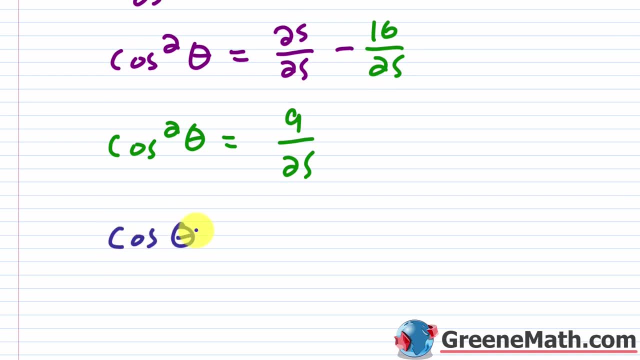 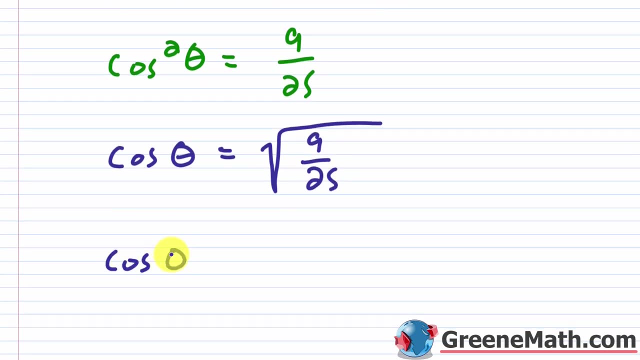 square root of this right hand side. So I'm going to say the cosine of theta is equal to the principal square root of nine over 25.. So now let's finish this up and say the cosine of theta is equal to square root of nine is three. 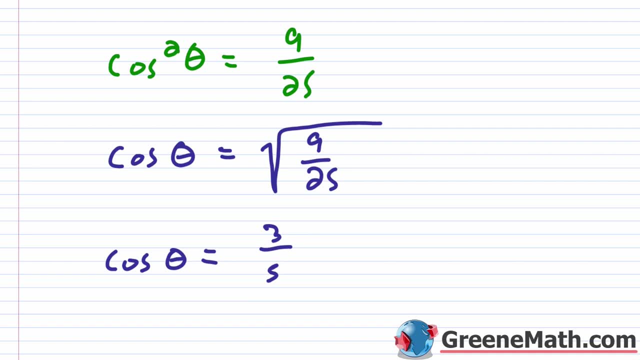 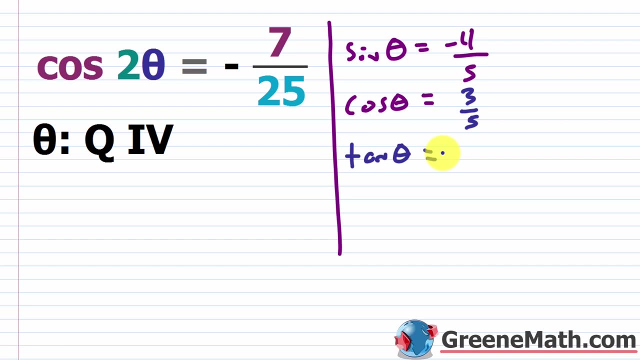 square root of 25 is five, So this is three fifths. So let's come back up And this will be three fifths. Okay, so then the tangent of theta is found by what you basically take this guy right here, this negative four fifths, and you multiply by the reciprocal of this, this five thirds. 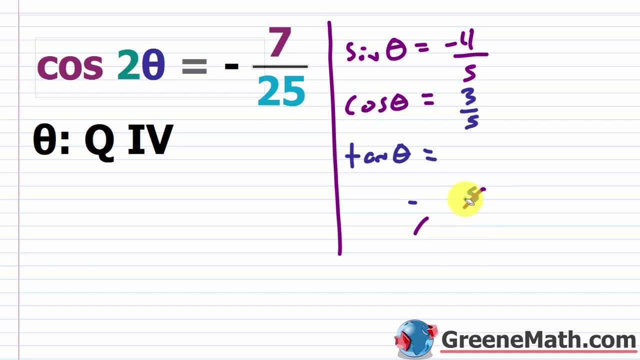 okay and this cancels and you get negative four thirds. So this is negative four thirds. And then the other guys are found, The reciprocal identities. So let's just go ahead and do the cotangent really quickly, So the cotangent of theta that's found by flipping this. so it's negative three fourths. Then, if I want, 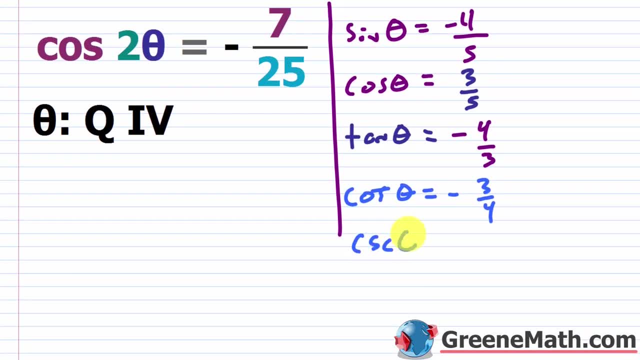 let me scroll down just a little bit. If I want the cosecant of theta that's found by flipping this, this sine of theta, So this is negative five fourths. And then, lastly, if I want the secant of theta that's found by flipping the cosine of theta, So that's going to be five thirds. 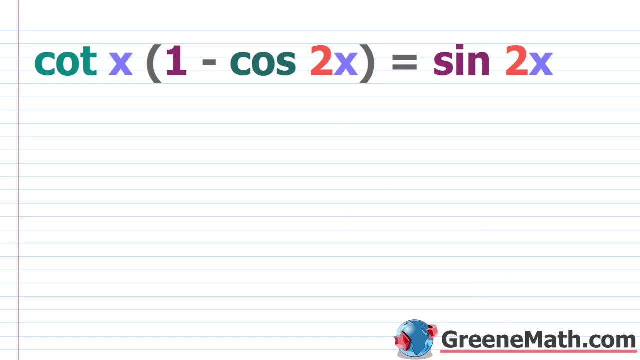 Okay, let's look at two examples of verifying some trigonometric identities. You always want to get practice doing this because it keeps coming up again and again and again, And the more you work on it, the better you're going to be when you need it for calculus. Okay, 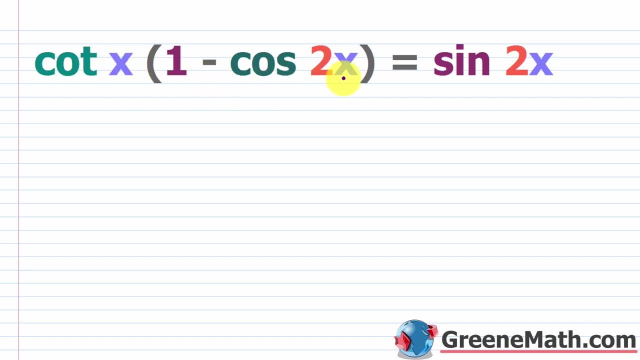 so we have the cotangent of x times the quantity one minus the cosine of two x is equal to sine of two x. So the first thing I'm gonna do is flip this. I'm going to put sine of two x here, basically on the left hand side for formatting, and I put is equal to. let's just go and put: 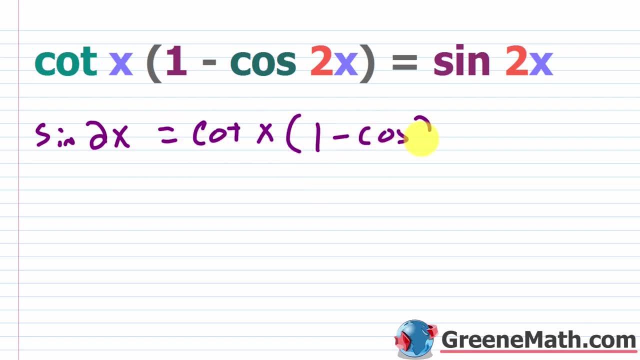 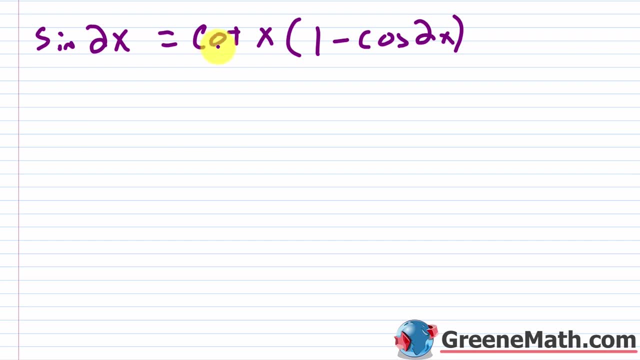 cotangent of x times the quantity one minus the cosine of two x. Okay, so how can we approach this problem? The first thing I always like to do if I see something like the cotangent of x or the tangent of x, the first thing I'll try. I'll try to put things in terms of 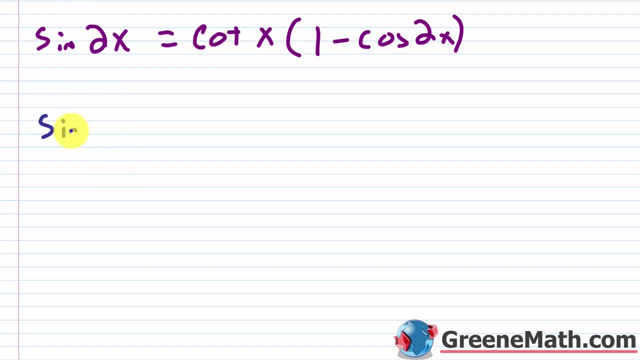 sine and cosine. It doesn't always work that way, But in this case it will work out this way. So we have the sine of two. x is equal to. I'm going to go ahead and say that the cotangent of x is the. 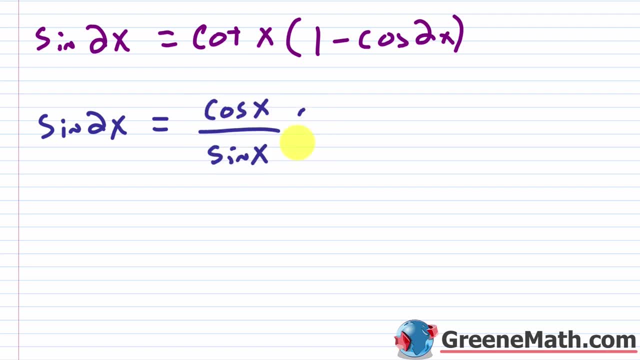 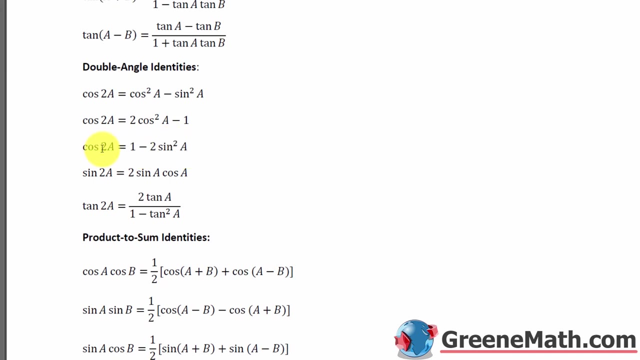 cosine of x over the sine of x, And this is times the quantity one minus the cosine of two x. Now you have one minus something and I want you to look at the identities here. If you go back here, notice you have this: one minus two times sine squared of a. here for the cosine of two, a. Okay. 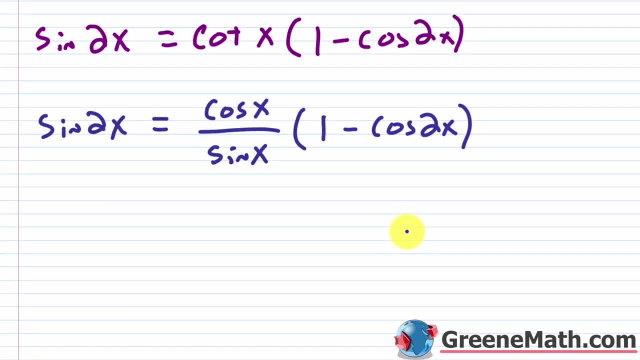 so if I plug this in here, I can get that one to drop out. So I'm going to go ahead and write this as the quantity. make sure you use parentheses here. one minus two times sine squared, in this case of x. Okay, so you need parentheses there because you're subtracting the whole thing away. 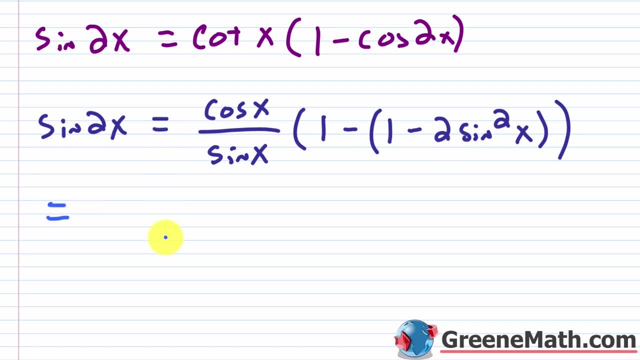 What I'm going to have here. my equals over here- and I know normally you line this up, but I want a lot of room So I got to do it over here. So cosine of x over sine of x times, in this case, you could go ahead and write this: 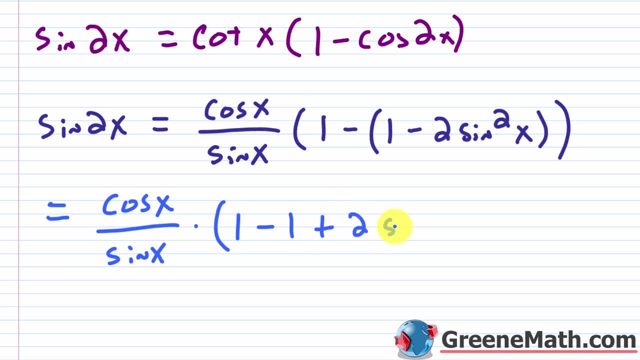 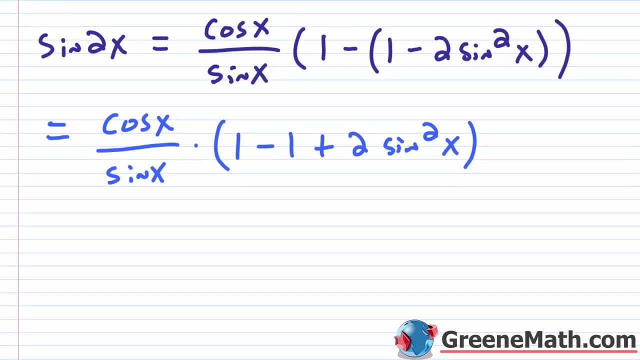 as one minus one plus two times sine squared x And see how the ones are going to cancel out there. So let's scroll down a little bit more, get some room. I'm going to say is equal to- I'm going to go- cosine of x over sine of x times one minus one is zero. 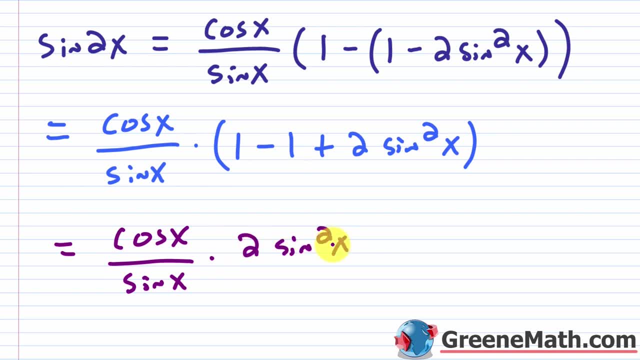 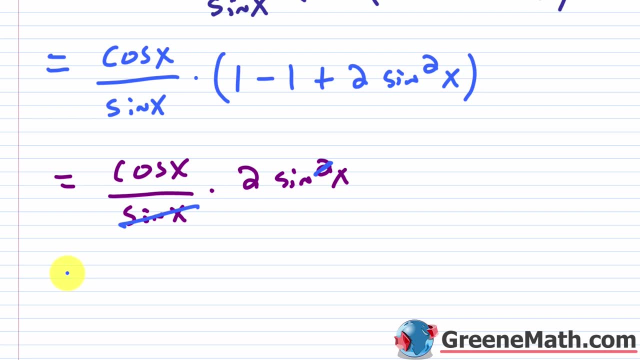 so that's gone. You have two times sine squared x. Now you can do some canceling, right? This is going to go away. I can get rid of one of these right. So basically what I can do here is say: 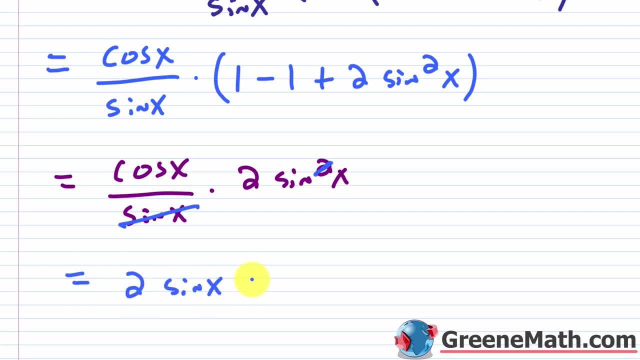 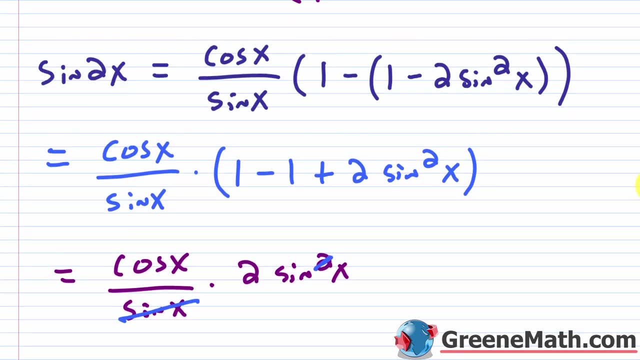 that I have two times sine of x, times the cosine of x. Now, let's stop for a minute. If we go back up, we're trying to get the sine of two x. Okay, so that's what we want. So is there an identity? 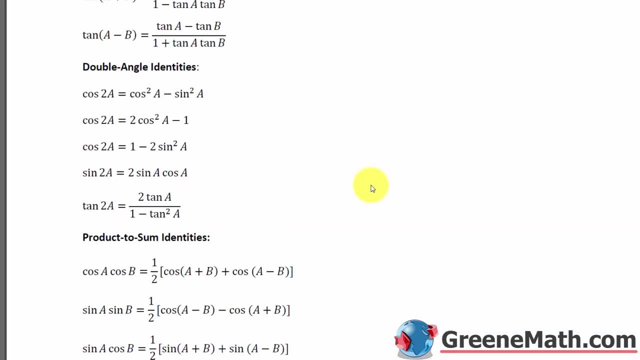 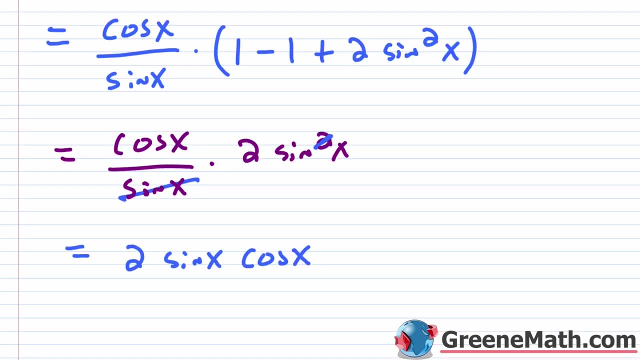 that matches that. If we go back, we have that the sine of two a is equal to two times sine of a times cosine of a. So we're basically done right. We can basically replace this right here with the sine of two x, So we can go ahead and put a big fat checkmark there to show that we're done Okay. 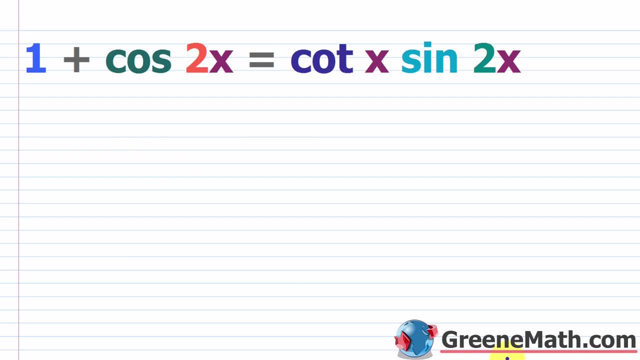 let's look at another example Again. I just want to do a lot, a lot of examples of these. So we have one plus: the cosine of two x is equal to the cotangent of x times the sine of two x. Okay, so which side is more simple? I would say that because this has cotangent involved. 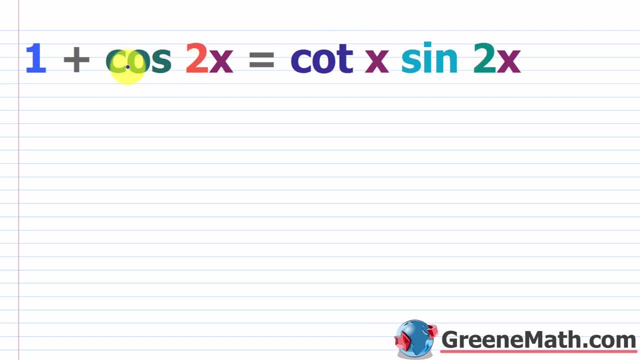 and this just has cosine. right, This is cotangent over here and you have cosine, So I would not mess with the left hand side, I would mess with the right hand side, So I would put equals over here And I would change this into again cosine. 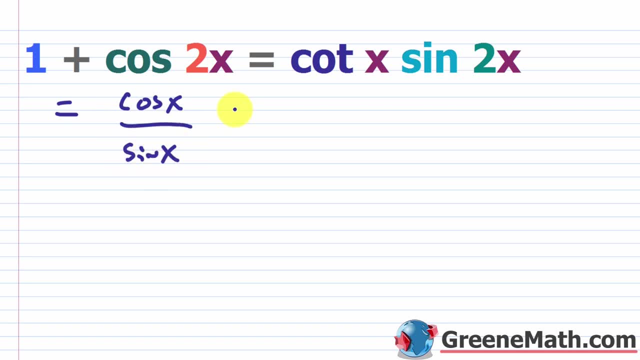 of x over sine of x, just to get started Again. it doesn't always work out that way. And then you have the sine of two x. So be careful here, don't go through and cancel this with this immediately, Because this is not like having sine squared of x, right, This is sine of two x. So you basically 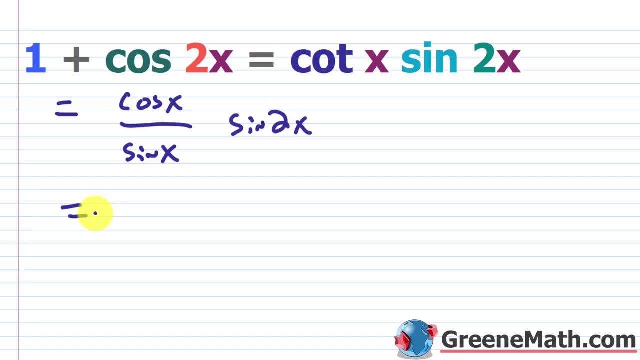 want to use your little formula where the sine of two times x is basically two times the sine of x times the cosine of x. So let's put cosine of x over sine of x And let's say basically over here we have, instead of sine of two x, I'm going to put times two times the sine of x times the. 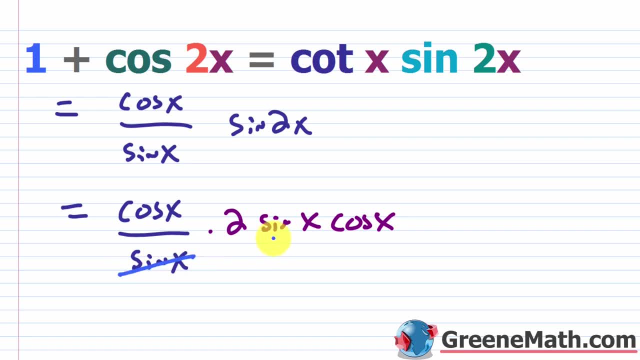 cosine of x. Okay, so now we can cancel this with this. Again, don't cancel it here. That's not correct. You have to cancel here when it's sine of x and sine of x, Or if you had sine squared of x. 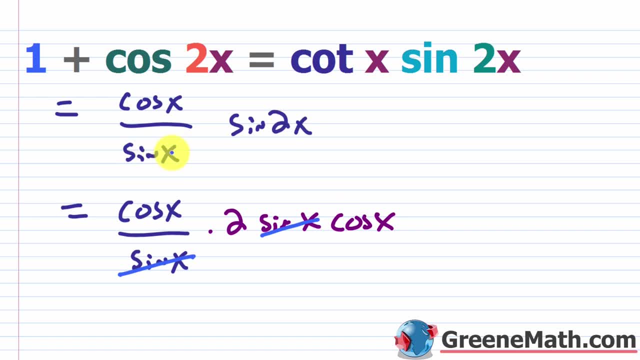 or something like that. then you can cancel. But sine of two x you're not gonna be able to cancel with sine of x. It doesn't work that way. So you're not going to be able to cancel with sine of x. 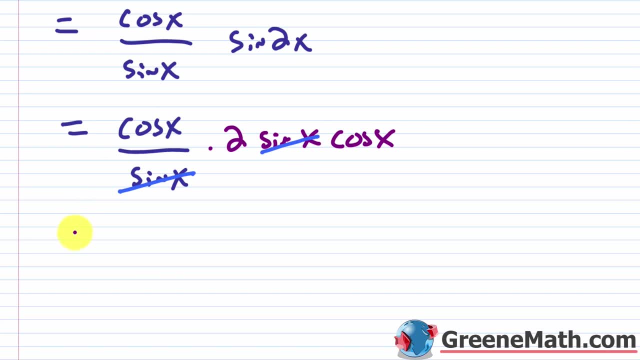 So let's come down here a little bit, Okay, And let's go ahead and put our equal sign And now basically what I'm gonna have is two times cosine squared of x. So you might think you have a little stopping point here, because I'm trying to get one plus cosine of two x. But again, if you look at, 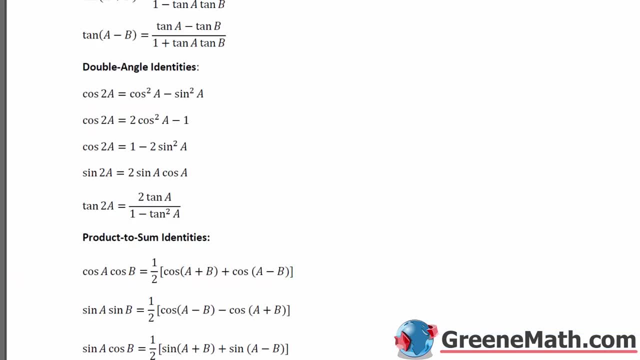 your identities, you're going to find something that can match. So if I come back here right now, we have two times cosine squared of x. Okay, If I add one to each side, it's exactly what I'm looking for, right? Cosine of two a plus one. 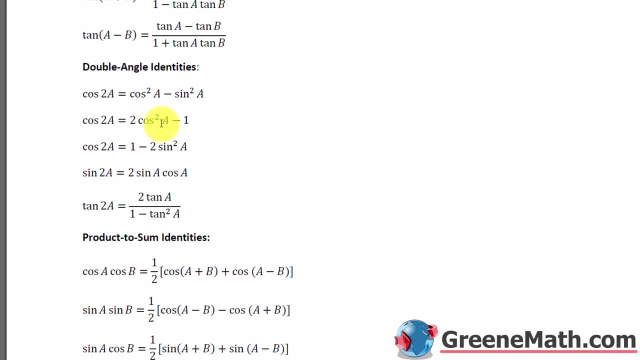 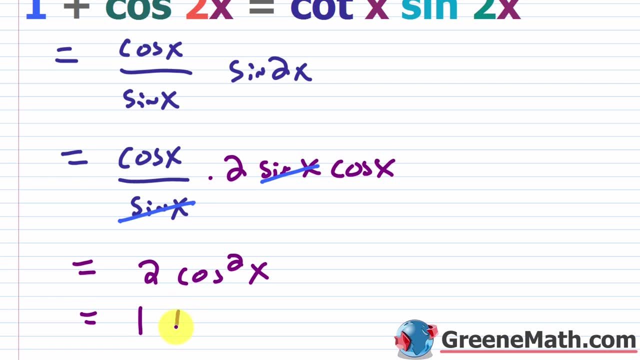 Is equal to two times cosine squared of a. Okay, So basically, I'm just going to replace this guy right here with its alternative form. I'm gonna say: this is equal to one plus the cosine of two x. Okay, So straight from your identities handout, we'll go ahead and put a check mark there. 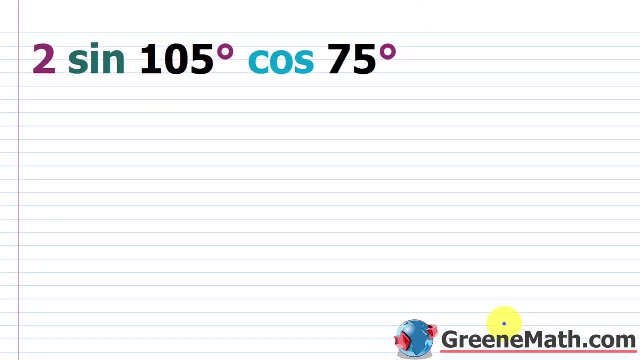 because we're done. Okay, Let's look at some problems that involve the product to sum identities and also the sum to product identities. These come in a variety of forms. Sometimes you're asked to find the exact value. Sometimes you're asked to simplify. These guys are. 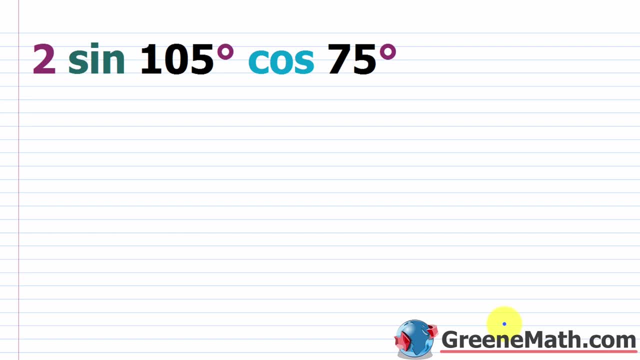 really, really easy to work with, As long as your teacher allows you to have the sheet in front of you. Otherwise, you do have to memorize. Okay, So what we have here is two times sine of 105 degrees, times cosine of 75 degrees. So, basically, this is a product, Okay, And we're going to want to change. 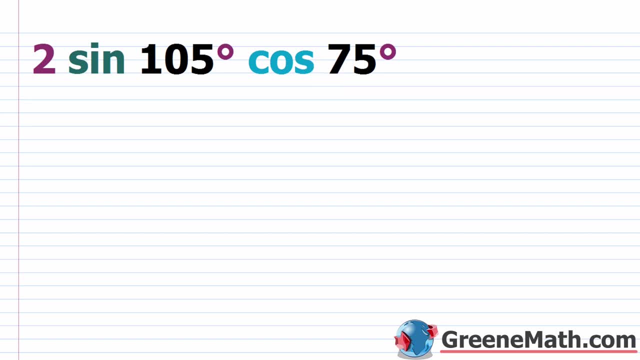 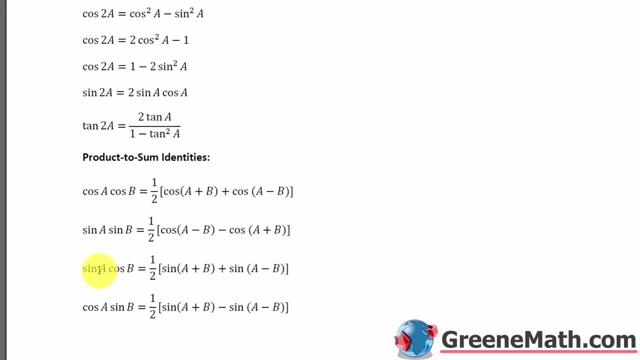 this into a sum to get an exact value. So let's go to our little worksheet here And there's quite a few of these, So let's go to basically where we have our sine of a times our cosine of b like this: This is going to be one half times cosine of b times cosine of a times cosine of b times cosine of b. 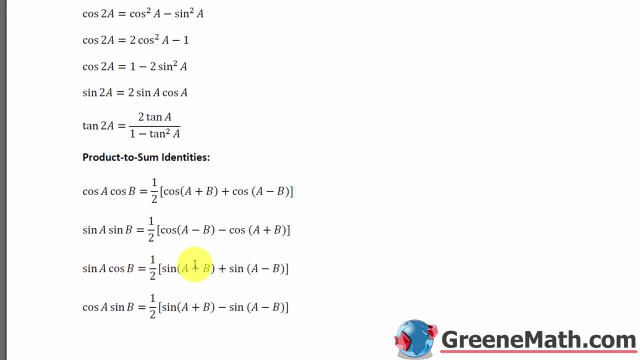 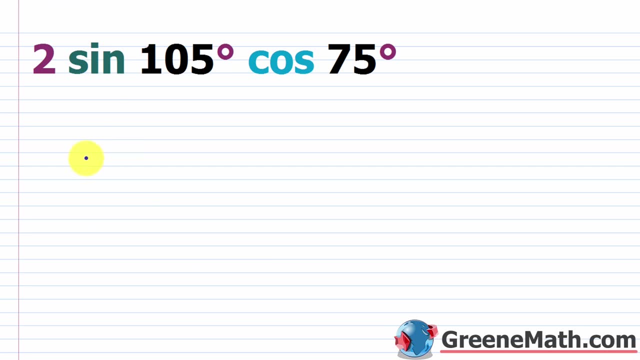 half times inside these brackets. here You have the sine of a plus b, plus the sine of a minus b. Okay, So let's just put this down here and I'll just write it out really quickly for you. So, basically, if we have the sine of a times the cosine of b, okay, which is what we have, right. 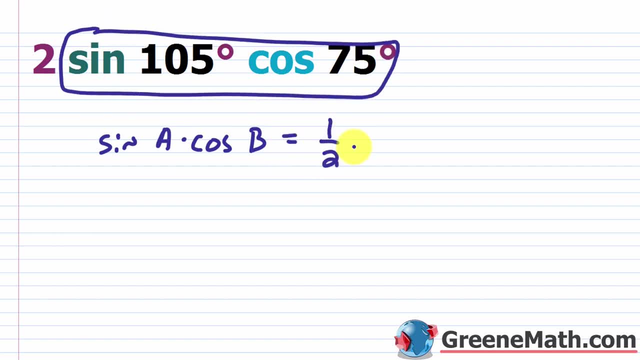 here, then basically, this is going to be one half times the sine of. let me put this in brackets: a plus b, Okay, And then you have your plus your sign of. let me slide this down. This is not going to fit. 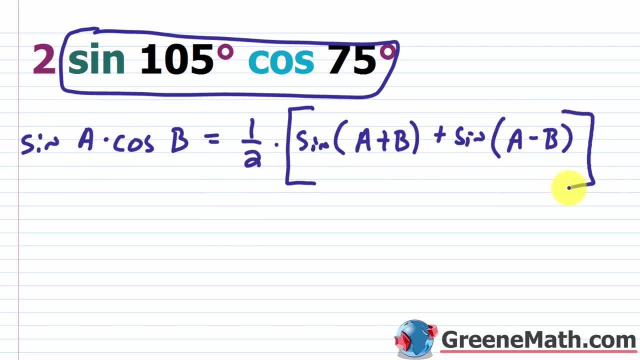 So your sign of your a minus b: Okay. So let's close that down. So the first thing is you can cancel this immediately by saying you have two times this one half here, or you can cancel later, It doesn't really matter. You can put this as two times and then you can put brackets here. 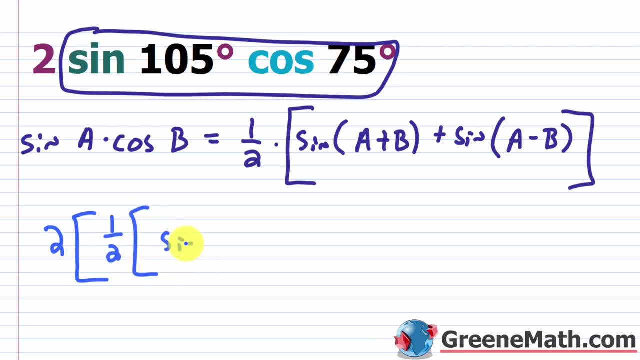 and then put one half and then put more brackets and then put your sine of what's a- in this case, that's going to be 105 degrees. What's b, That's 75 degrees. so 105 degrees plus 75 degrees is 80 degrees. okay, let me just write this like this. i'll just put sign. 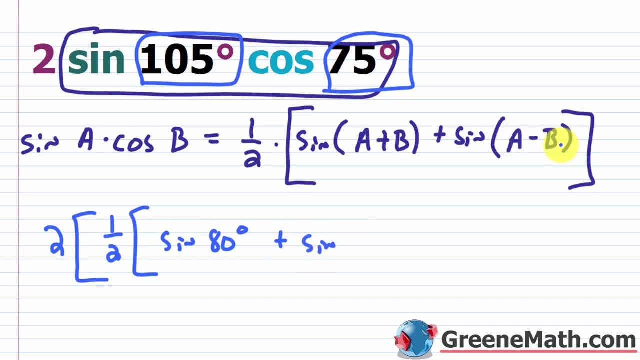 of 80 degrees, plus the sign of what's a minus b, what's 105 degrees minus 75 degrees, that's going to be 30 degrees. okay, so you can put these brackets here again, it's not going to matter, because when two gets multiplied by a half, it's basically going to be one, right? so it's basically. 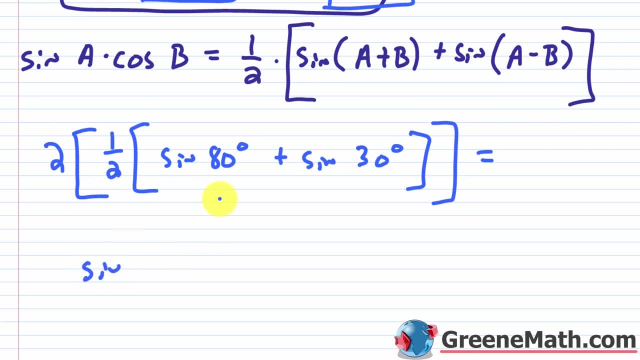 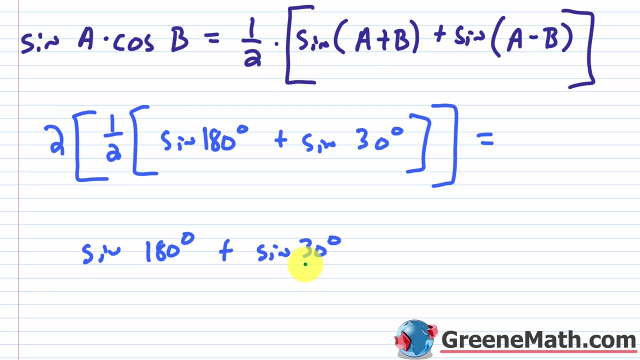 gone. so we can just say that we have the sign and i put 80 degrees, this should be 180 degrees, so the sign of 180 degrees plus the sign of 30 degrees. so at this point you should be very familiar with your unit circle. the sign of 30 degrees, you should know, is one half and the sign 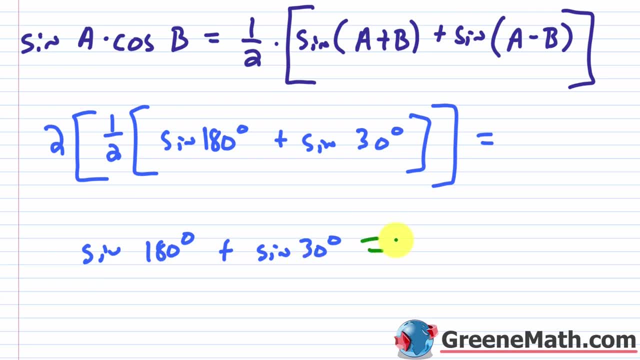 of 180 degrees, you should know, is zero. so this basically turns into zero plus one half, which gives me one half. okay, so just a little formula where you start off with something that looks kind of hard to work with. you plug some things into the formula and you get an exact value of 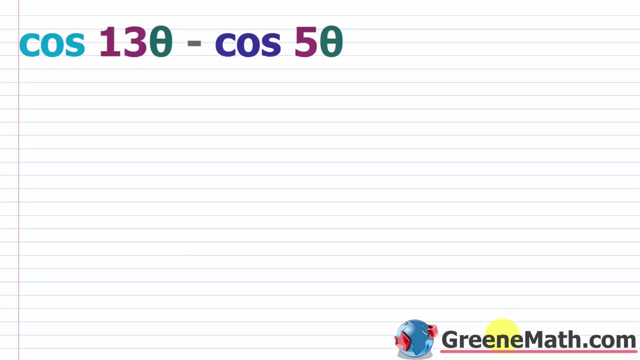 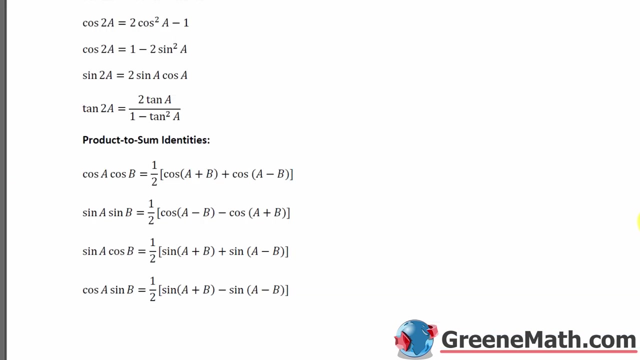 a half. okay, let's look at an example of what we call a sum to product here. we're just going to be asked to simplify. so you have the cosine of 13 theta minus the cosine of 5 theta. okay, so basically we want to change this into a product. so let's go ahead and go back and look at now if we come. 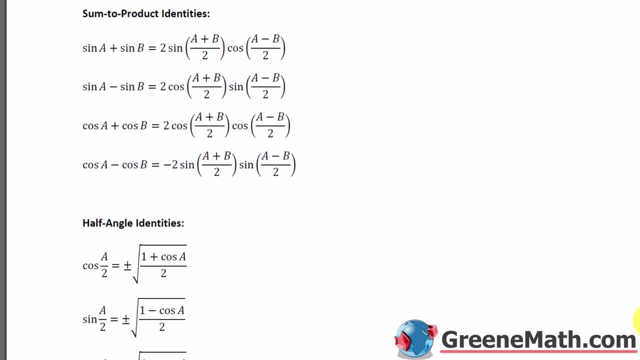 down here. we have the sum to product identities. we have the half angle identities, but we'll get to that in the next lesson. so what we have here is cosine of sum a minus cosine of sum b. this equals negative: 2 times the sine of this a plus b over, 2 times the sine of this a minus b over. 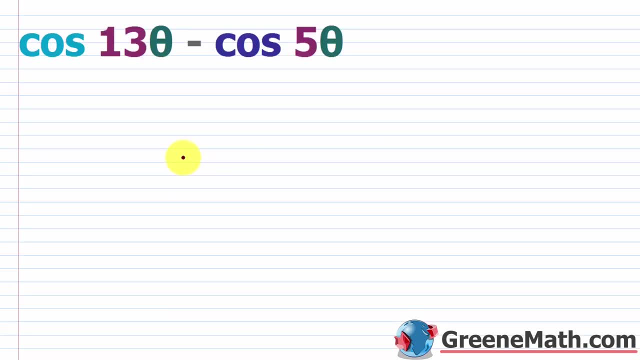 2. okay, so let's go back and let's just write this down here. so basically, the cosine of a, okay, minus the cosine of b is equal to negative, 2 times the sine of you. have this a plus b over 2. okay, times the sine of you have this a minus b over 2. okay, so i'm just going to plug in: a is going to be 13 theta. 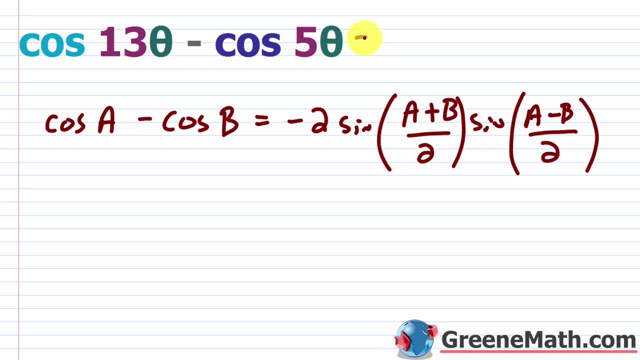 plus 5 theta. okay, so let's think about this. i'm going to put equals and i'm going to carry this over here and let's just go ahead and say that we have negative 2 times the sine of what's a plus b. well, it's 13 theta plus 5 theta, so that's going to be 18 theta over 2. okay, so i can go ahead and 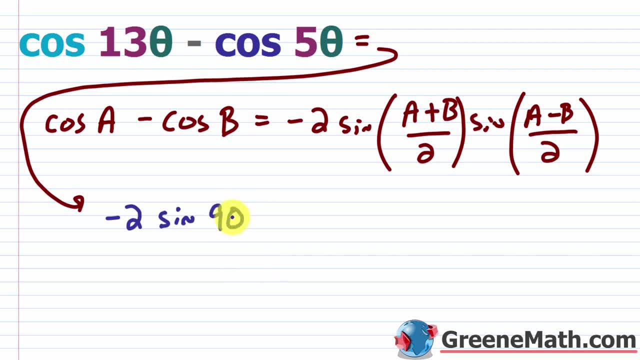 reduce that and say that's basically 9 times theta. right, so sine of 9 times theta. and then now, so 13 theta minus 5 theta is going to be 8 theta. okay, over 2. again, 8 divided by 2 is just 4. 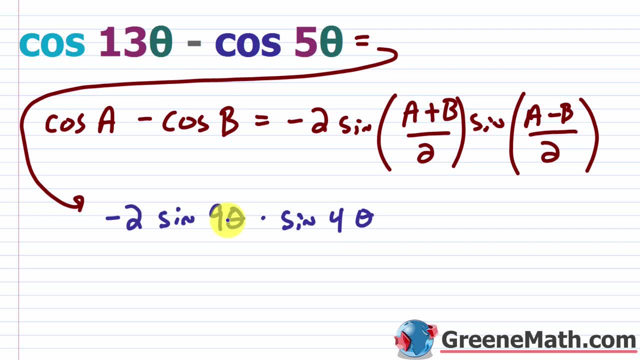 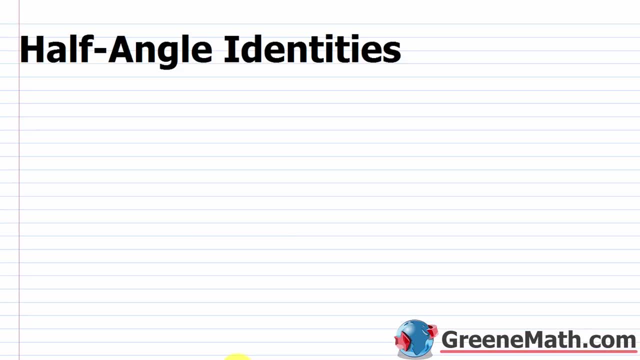 so you can put that like that. that's basically all we can do if we're asked to write this as a product. so we have negative 2 times the sine of 9 theta times the sine of 4 theta. in this lesson we want to talk about the half angle identities. all right, so we're going to wrap up our section. 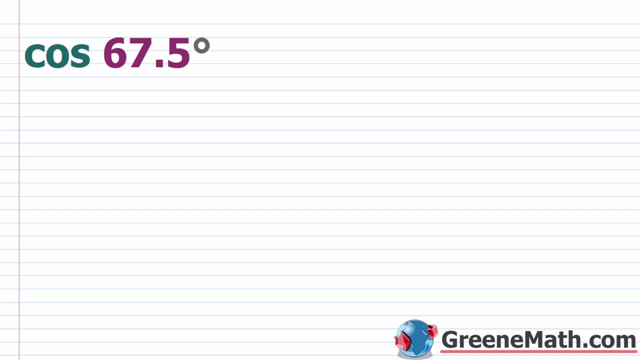 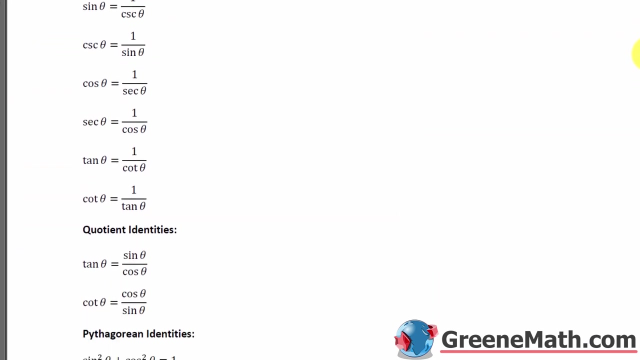 now on the trigonometric identities and get ourselves prepared for solving trigonometric. we need to talk about these half angle identities. so let me quickly go back to our handout. so we have all of our trigonometric identities listed here, so these are the ones we've already. 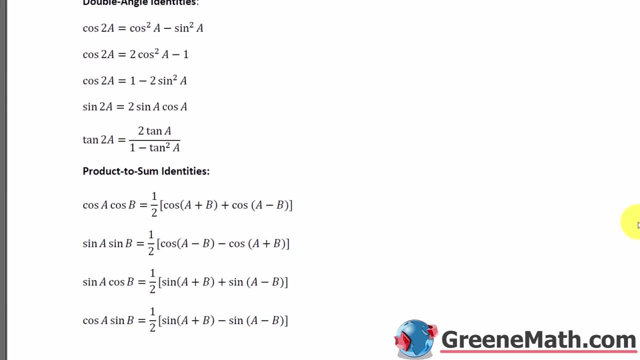 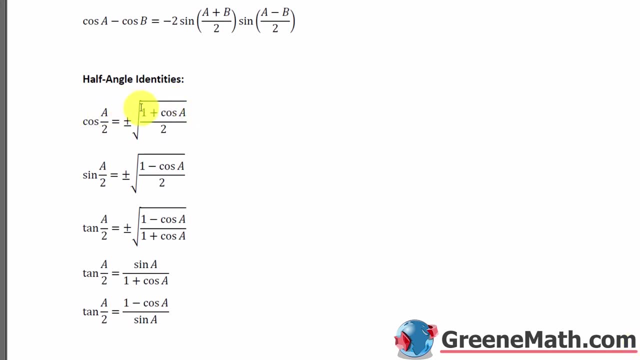 talked about. let me just keep scrolling down here. we're going to come down to all the way down where we have these half angle identities. okay, so you see, you have ones for cosine sine, you have three for tangent- again something you need to basically memorize if you want to go quickly through these. 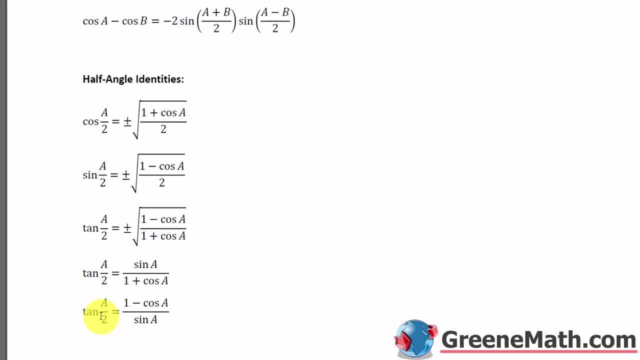 problems, but in a lot of cases they're going to let you know that you're going to have to have these handouts, so it's something you could just refer to back and forth. okay, so i'm going to come back to these when i need them. the first one i'm going to need is this guy, so you can pause the. 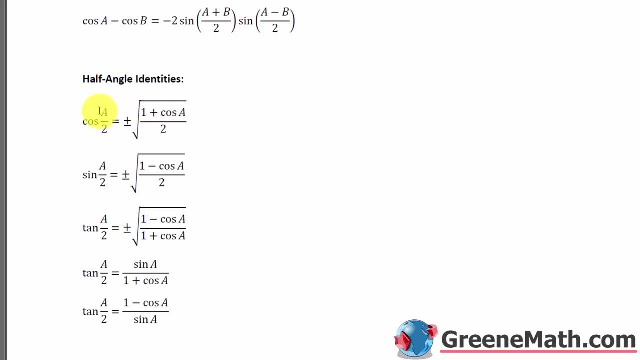 video and write it down, or you can have your handout, whatever you want to do, but the cosine of some angle, a over 2, is equal to, plus or minus, the square root of 1 plus the cosine of a over 2. now this plus or minus here is there to tell you that you want to take the appropriate sine based. 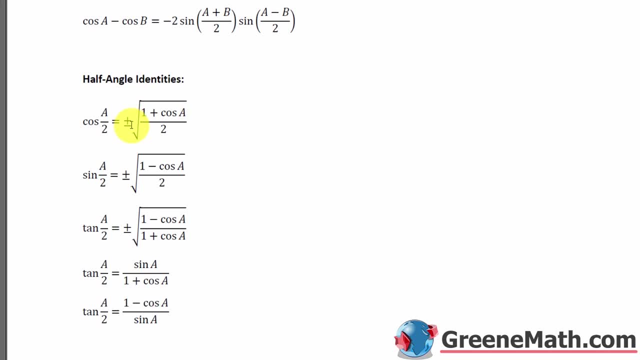 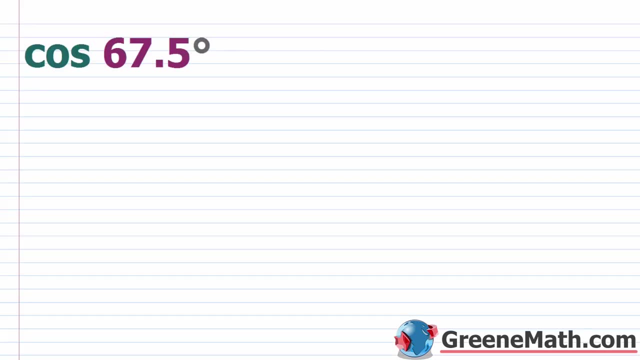 on the quadrant that you're in. remember, cosine is going to be the cosine of the square root of the positive in quadrants 1 and 4. okay, so let's go ahead and minimize this. let's go to the first problem here, where we're told to find the cosine of 67.5 degrees. now, before i start, let me just put. 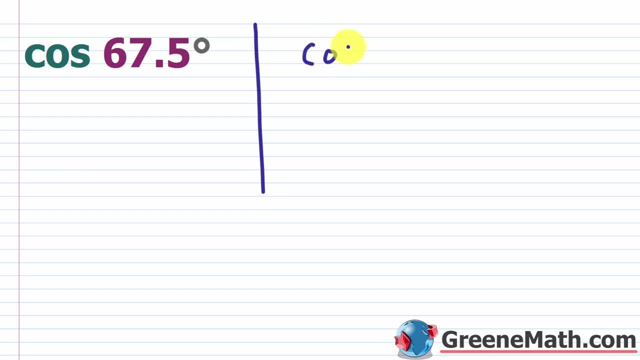 this off to the side. let me put my identity here. so the cosine of, let's say, a over 2 is equal to. we have plus or minus. you have the square root of. you're going to do 1 plus the cosine of this, a over 2. okay, so let me just slide this down just a little bit. so this is what we're going to be using. 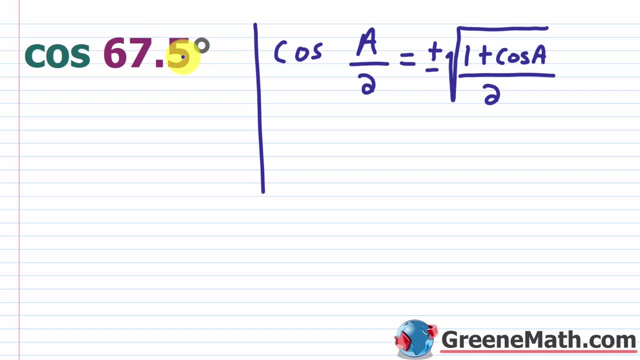 here. so basically, if i want to write this angle here as some angle over 2, i would first multiply by 2 to figure that out, right? so 67.5 times 2 is going to give me 135, right? so i would say this is equal to the cosine of 135 degrees over 2. okay, so now this guy right here matches my format. 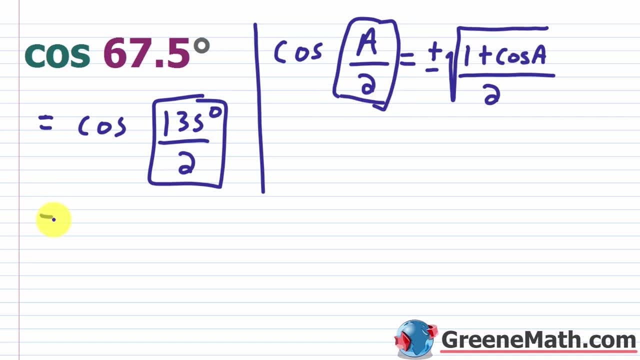 right here. okay, so i can use my little cosine of 135 degrees over 2 and i'm going to take this little identity here. so let's just put equals here, and i'm going to put, since we're trying to find the cosine of 67.5 degrees. remember, it has nothing to do with this guy that's being divided. 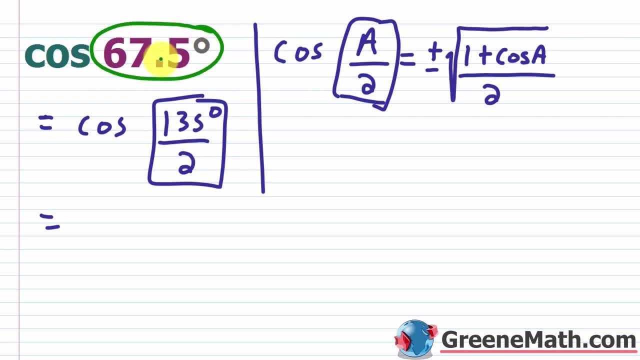 by 2. this is what we want here. okay, so this angle right here is going to be in quadrant 1. so we know cosine is positive in quadrant 1, so we want to use the principal square root. so i'm going to say this is equal to the principal square root of 1 plus the cosine of here's where it gets. 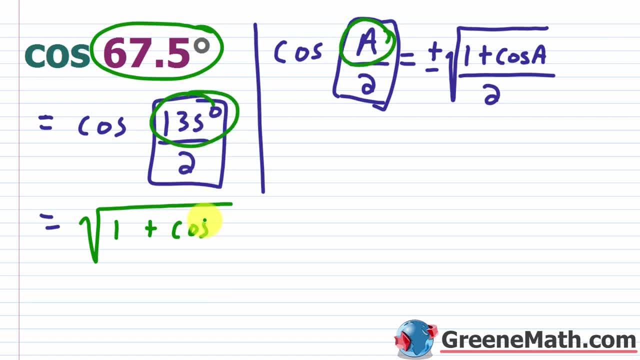 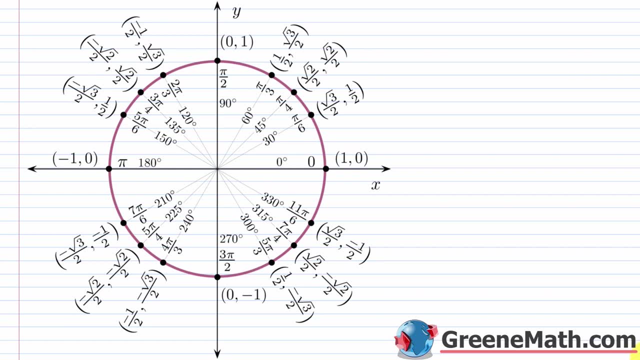 tricky. this is a. this is a. okay. so you want the cosine of 135 degrees and then over 2- okay. so this is what we're going to be figuring out now. hopefully at this point you've memorized the unit circle, but if you haven't, i have it here. so, basically, 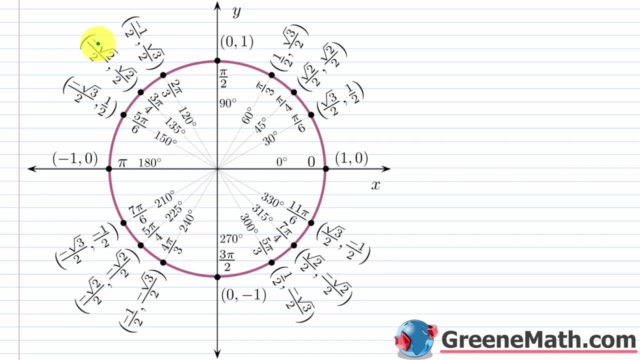 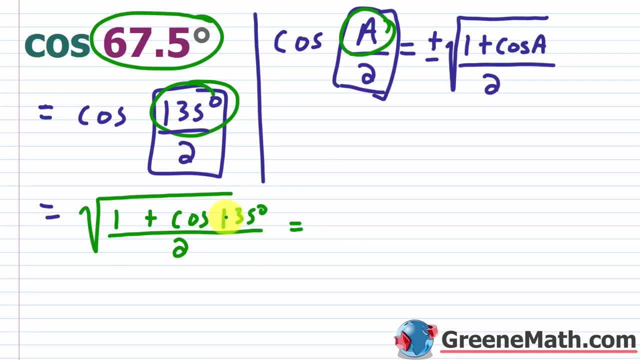 if you go to 135 degrees and you look at your x coordinate here, this is going to be the cosine of 135 degrees. so you have negative of the square root of 2 over 2 and all we need to do is replace that here. okay, and once you have that, it's basically just a lot of simplifying, okay, so 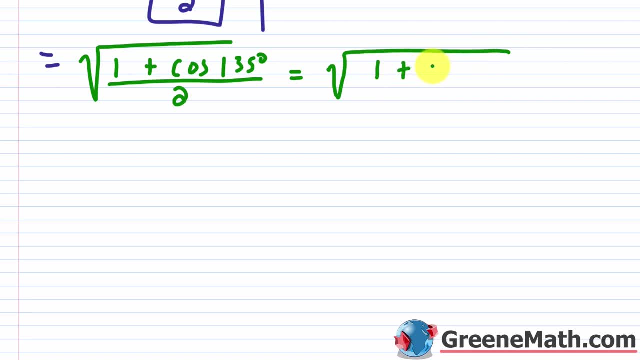 let's just put the square root of 1 plus again. this is the square root of 1 plus, and then we're going to put the negative of the square root of 2 over 2 and then all over 2, and i should probably make this a little bit bigger so it encompasses the whole thing. let's continue this over here. 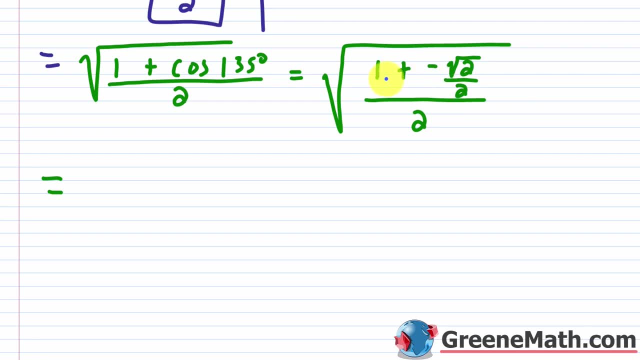 so the quickest way to do this, in my opinion. you could get a common denominator there. but i'm just going to multiply by 2 over 2. okay, so 2 times 1 over here would be 2. let me make my square root symbol. and then 2 times you'd have negative square root of 2 over 2. the 2s would cancel. 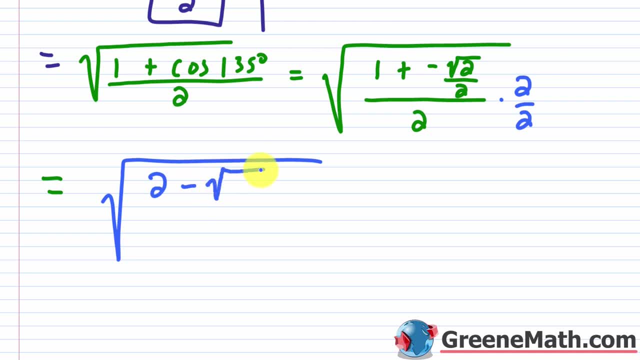 so you're basically subtracting away the square root of 2, so i'm going to put minus the square root of 2 and this is over 2 times 2. here is 4. okay, so we can quickly simplify this by realizing again: you could write this as the square root of 2 minus the square root of 2 over the square root. 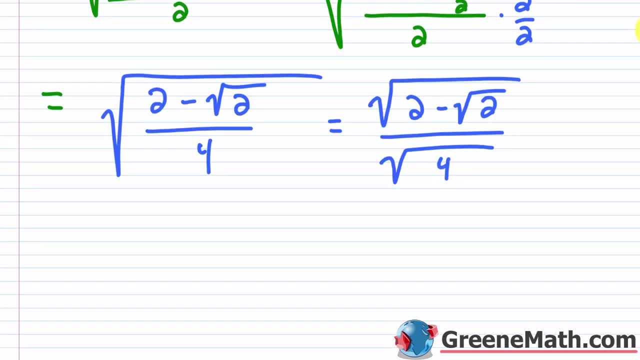 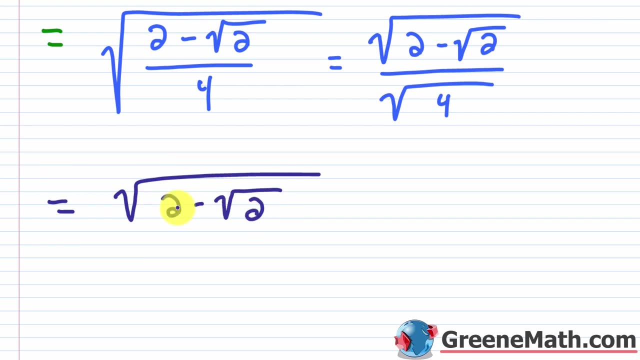 of 4. we know the square root of 4 is 2. okay, so i can come down here. let's finish this up and just put: this is equal to the square root of 2 minus the square root of 2. you can't really do anything. 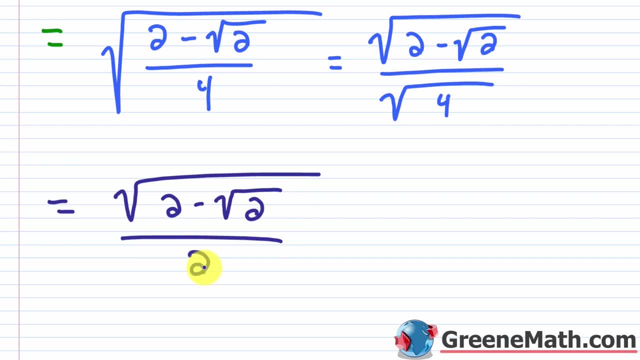 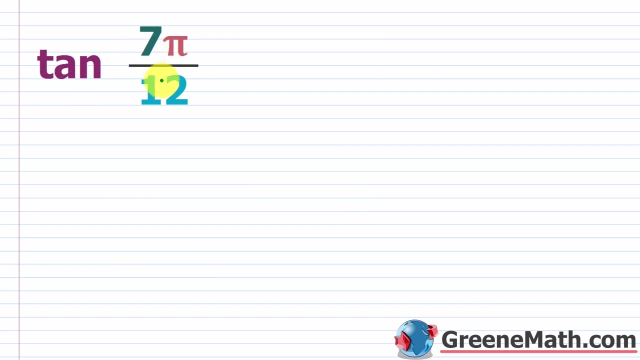 else there over the square root of 4 is 2. okay, so that's going to be your exact value. if you're for the cosine of 67.5 degrees, all right, let's take a look at a similar problem. now we're going to have the tangent, so we have the tangent of 7 pi over 12, and for this one again, if you get, 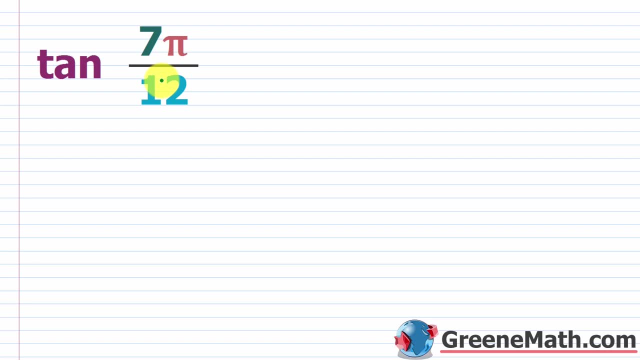 radians. if you're really good at working with fractions, you can do it in this way. i always just convert these into degrees because it's just easier for me. okay, so i'm going to first say: we have 7 pi over 12 times. again, to convert this, you want to put pi in the denominator. you want to? 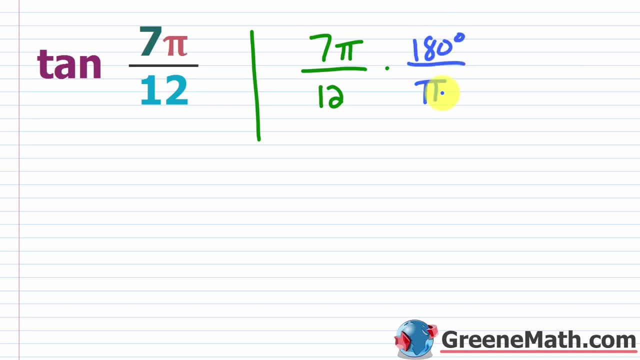 put 180 degrees in the denominator, so you're going to have the negative side of this and you're going to have the tangent of 7 pi over 12 times, so you're going to have the tangent of 7 pi over 12, the numerator. always remember that 180 degrees equals pi radians. okay, so this is your unit. 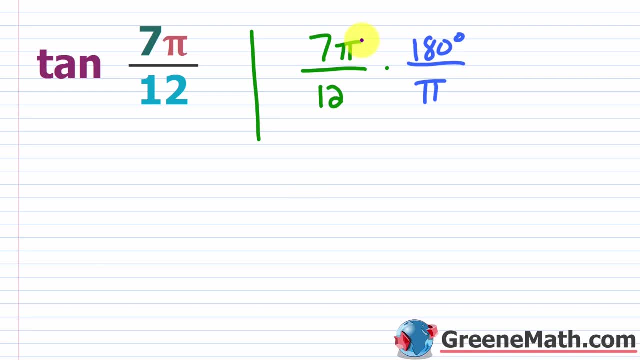 fraction, it's basically equal to one and we can use this to cancel. so this cancels with this. and 180 divided by 12 is 15, okay, so you can just cancel this out. put 15 15 times 7 is 105, okay, so. 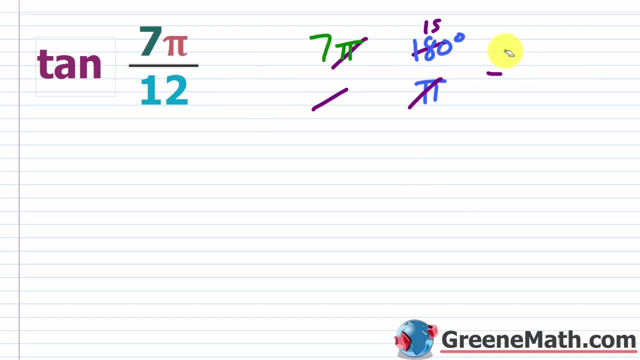 this will end up giving me 105 degrees. so let's erase this real quick and i'm just going to put that this is equal to the tangent of 105 degrees, and then i'm just going to double this number. okay, because i'm going to use this half angle formula. so i'm going to say this is equal to: 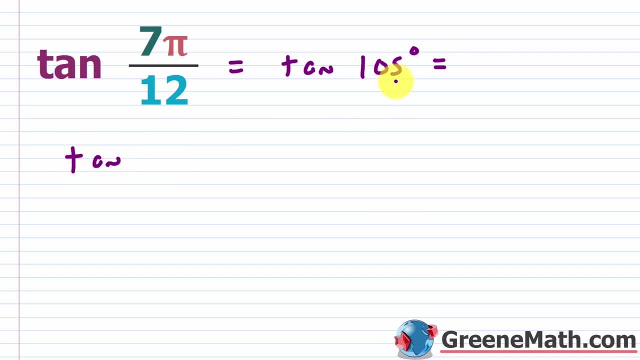 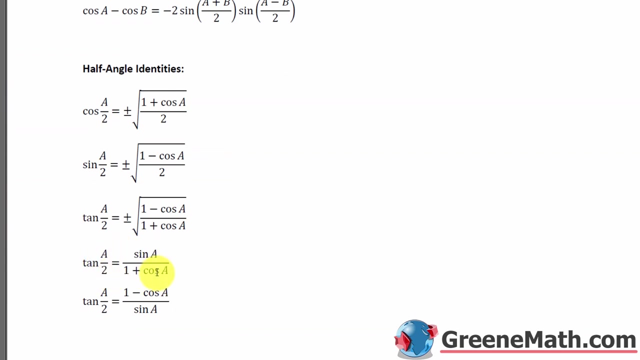 the tangent down here of 105 degrees times 2 is 210, so 210 degrees over 2. okay, so which formula do we want to use? let's go back to our worksheet, so you have several here to choose from. you can pick this one right here. i think it's probably the easiest. the tangent of a. 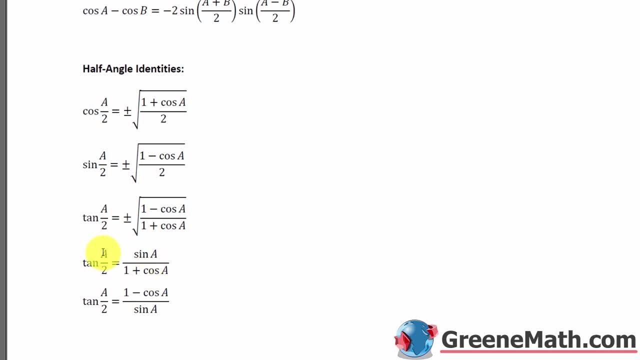 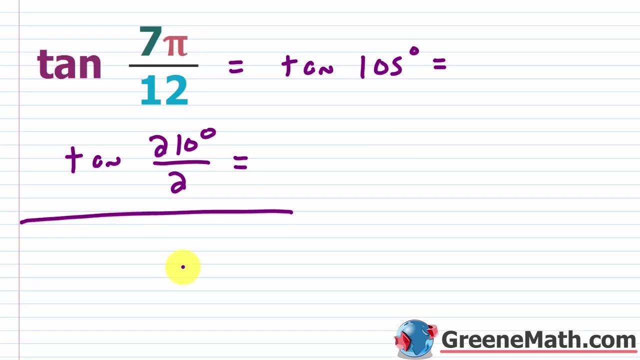 over 2. there's no square root symbol to work with. it's the sine of a, so the sine of whatever this is up here, over 1 plus the cosine of a. so let's go ahead and write this, maybe off to the side. we have that the tangent of a over 2 is equal to, again, this is the sine of a over you have 1 plus. 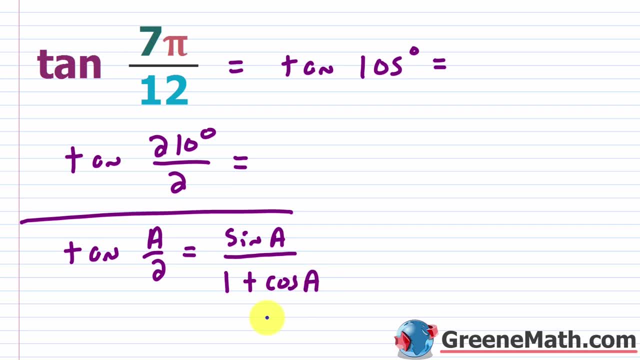 the cosine of a. so what do i want to do here? again, this is going to be what i'm plugging in for a here and here and here, okay. so basically i would say: this is the sine of 210 degrees over. you have 1 plus the cosine of 210 degrees, okay. 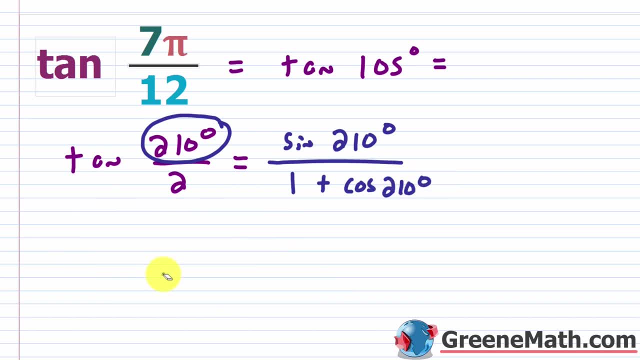 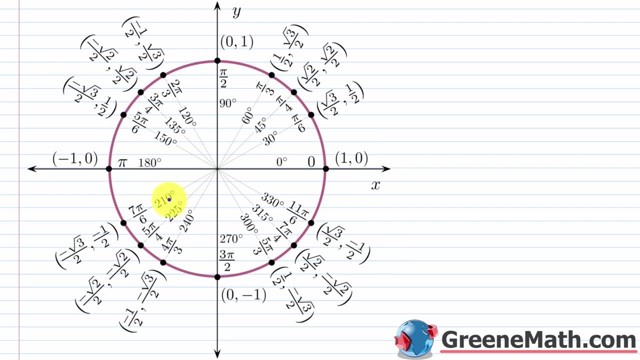 so we don't need this anymore. i'm just going to erase it for room, okay, and then i'll just put equals here. what is the sine of 210 degrees? let's go back to our little unit circle. so you have: the sine of 210 degrees is negative one half and you have the cosine of 210 degrees is negative square. 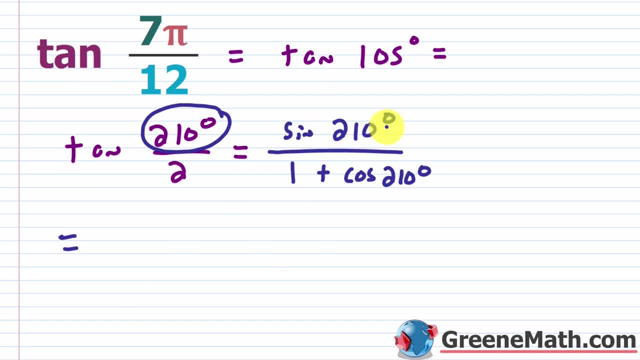 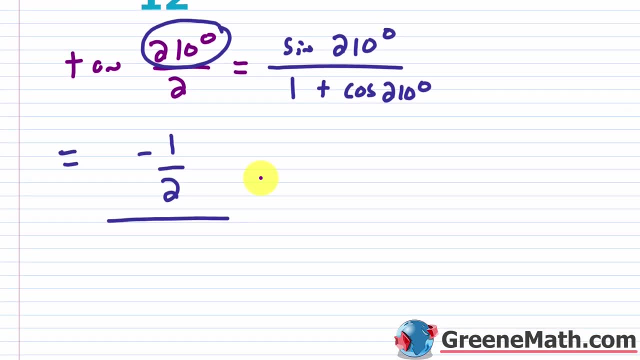 root of three over two. so let's now plug in. so the sine of 210 degrees is negative square root of one half. and then this is over. let me scroll down and get a little bit of room here. so again, this is over one plus. what's the cosine of 210 degrees? it's the negative of the square root of three over. 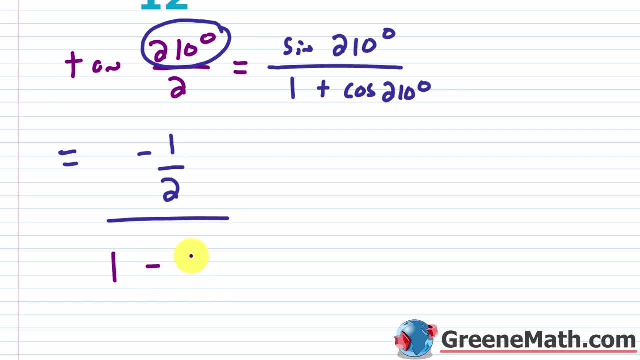 two. so let me put minus here instead of plus. so the negative of the square root of three over two. okay, so now all we really have to do is simplify this guy pretty easy overall. i'm just going to multiply the top and bottom by two. so this gives me what this is going to cancel. right, the twos would. 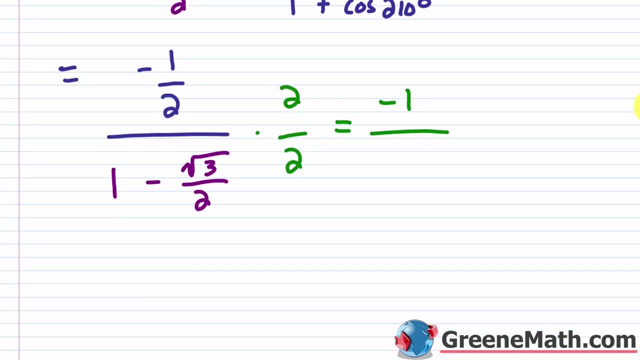 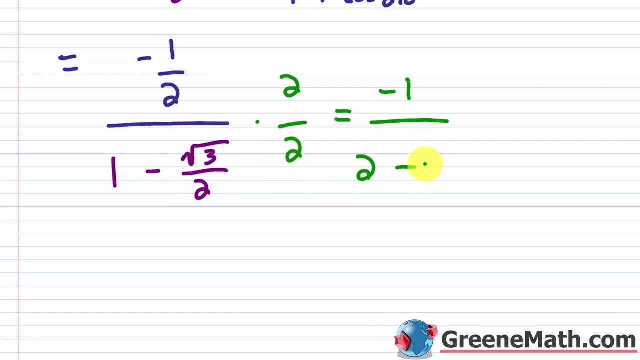 cancel and i just have negative one up here, and then this is over down here. two times one is two, and then minus two times this guy right here, the twos would cancel and you would just have the square root of three. okay, now you don't want to leave this this way, because you don't ever want. 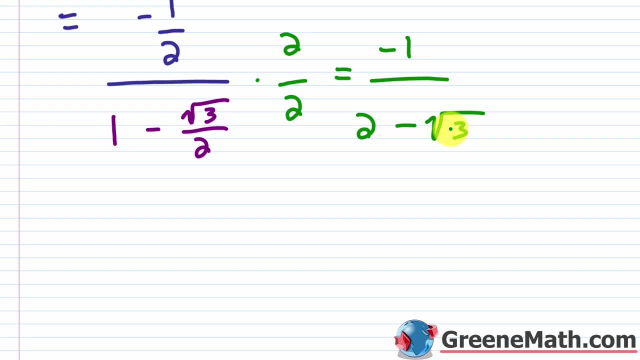 a radical in the denominator. so you need to rationalize the denominator. so let's put equals over here and i'll put negative one over two minus the square root of three. okay, remember how to rationalize this. when this guy is basically two terms, you want to use the conjugate right, so the terms would be the same, the two would be the same and 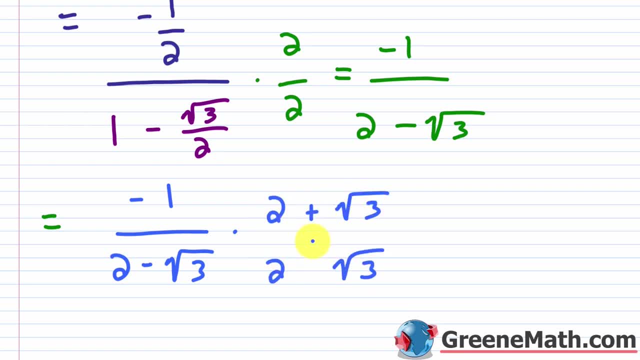 the square root of three would be the same, but you're going to choose the alternate sign. okay, and the reason for this is when you go through and do the foil down here, you're going to have those middle two terms drop out. so you're just going to have the first guy squared, minus the. 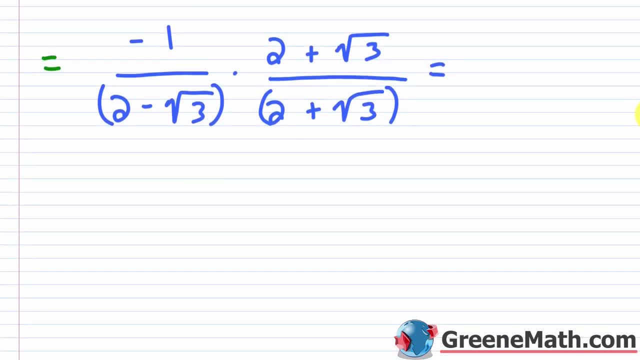 second guy squared. okay, so let's go ahead and put equals here in the numerator. we know what this is going to be: it's just going to make everything negative. so it would be, let's say, negative two. then minus the square root of three down here, you would have the first guy squared. so two squared is four, and then minus the last guy. 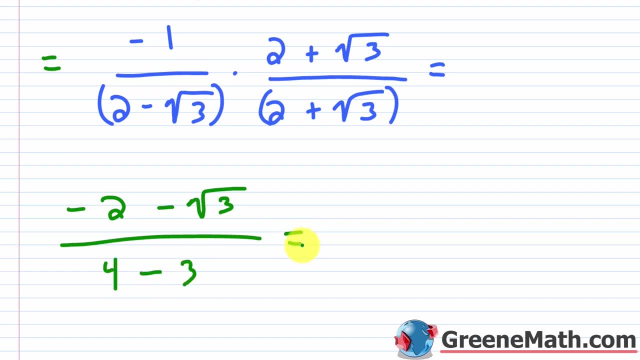 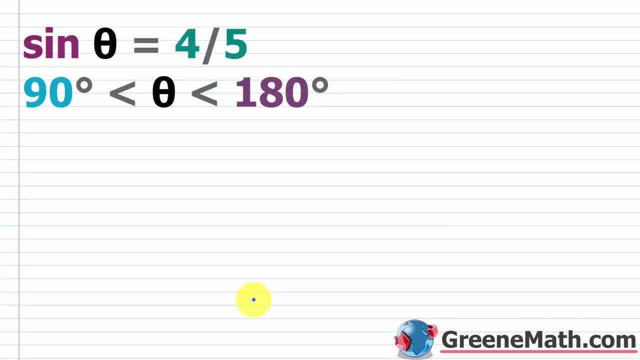 squared, which would be three. well, four minus three is one. so basically anything over one is just itself. so i can just say the answer here is negative, two minus the square root of three. all right, let's take a look at another common problem for this section. so your book will. 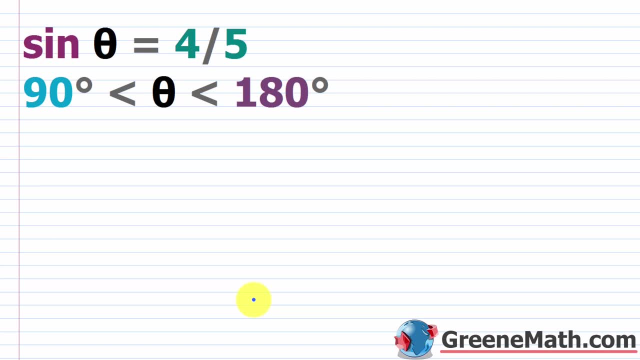 probably say something like finding function values of s over two, given information about s okay. so in this particular case, we are given that the sine of theta is four fifths and theta is basically in quadrant two right because it's greater than 90 degrees and less. 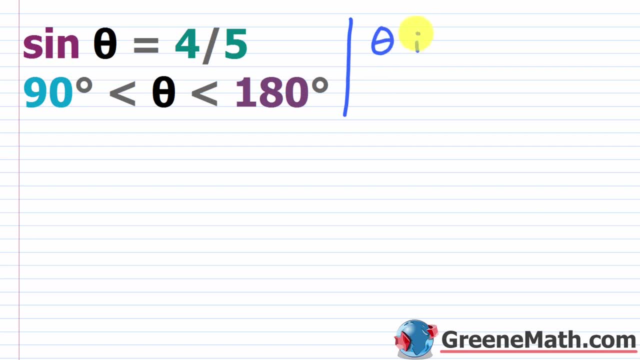 than 180 degrees. so you can basically say that theta is in quadrant two. okay, so we have that information. now what if i asked you to find, let's say, the sine of theta over two? and then let's say we want the cosine of theta over two and also the tangent of theta over two, and of course you can. 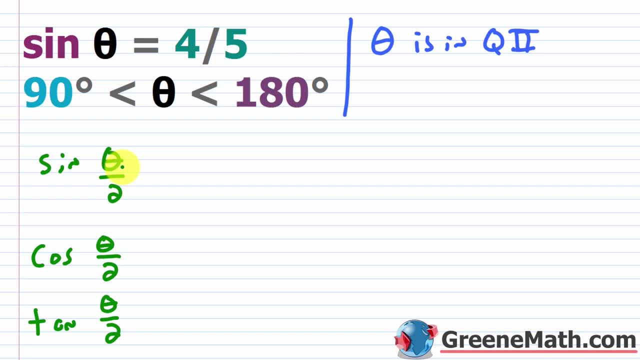 get the other ones with the reciprocal identities. we're just going to do these three because once you have those, you get the other ones easily, okay, so, first and foremost, where is theta over two? so theta over two is in what quadrant? so this is very confusing for a lot of people. 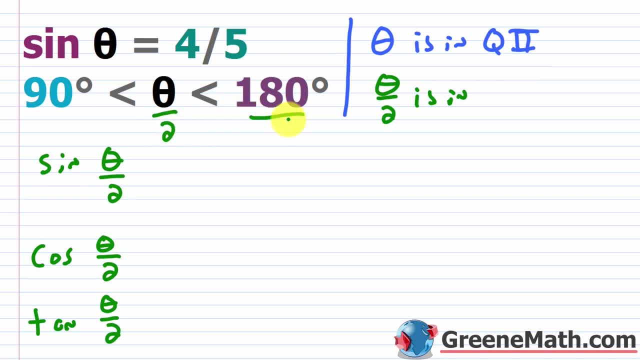 but basically, to determine this, you would just divide everything here by two. okay, because that would give you theta over two. now, 90 degrees divided by two is 45 degrees. okay, so that would be less than theta over two, which is also less than 180 degrees. divided by two would be 90 degrees. okay. 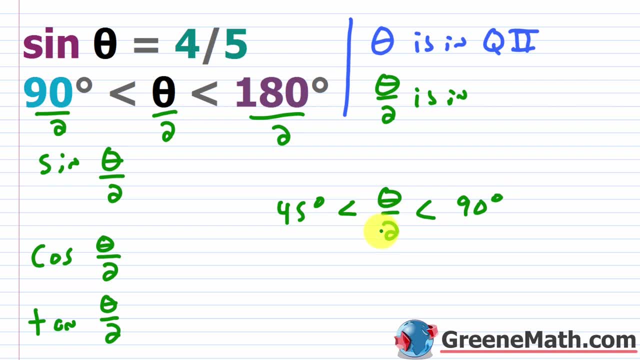 so this tells me that theta over two is greater than 45 degrees and less than 90 degrees. so it's got to be in quadrant one. so it's in quadrant one. so keep this in mind when you're working with these guys, because you've got to choose the appropriate sign. okay, for your trigonometric. 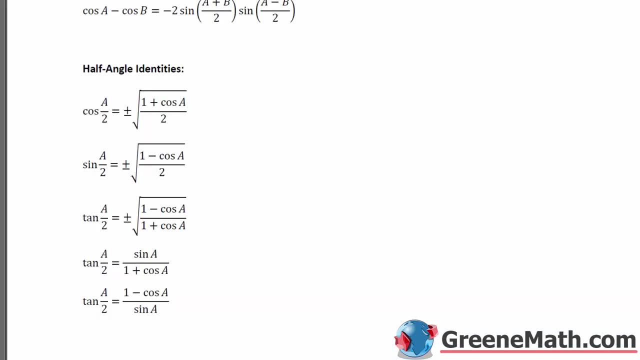 functions. now, if we go back to our identities, you'll see to find cosine of a over two or sine of a over two, you need to have the cosine of a, okay, in each case. so that means we first need to find cosine. so let me go to a fresh sheet and i'm going to go ahead and do that and i'm going to go. 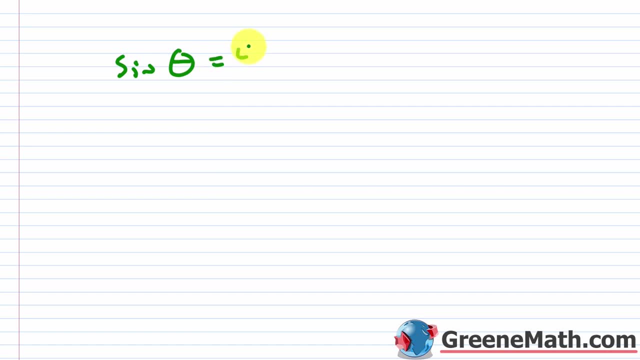 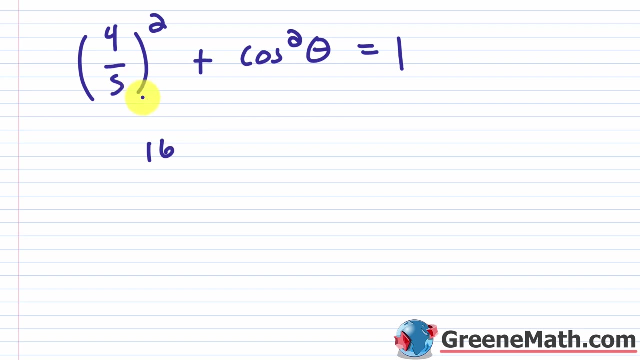 here and find what cosine square one is. 같아요 between four and theta. so basically that's the competitors who varían is equal to. i'm expecting fourth and fifth, because there's strong ят go to 1.. I'm going to subtract this away from each side of the equation, So this is going to be my. 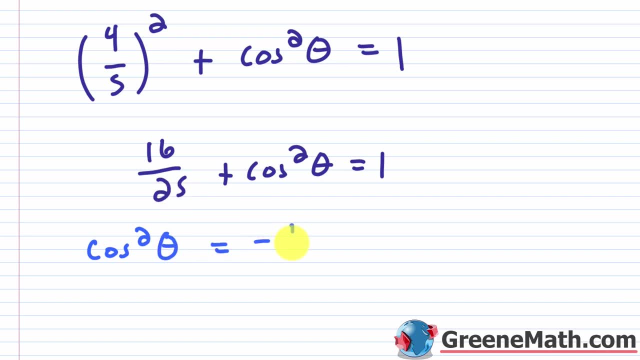 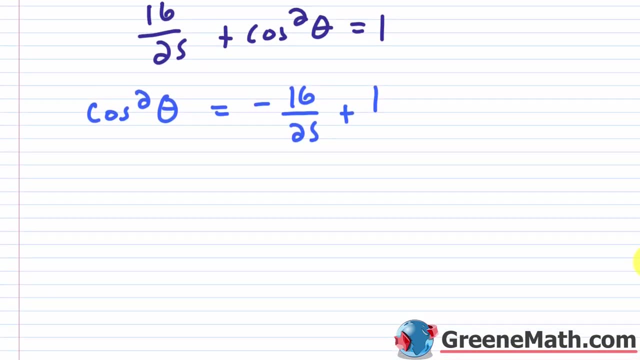 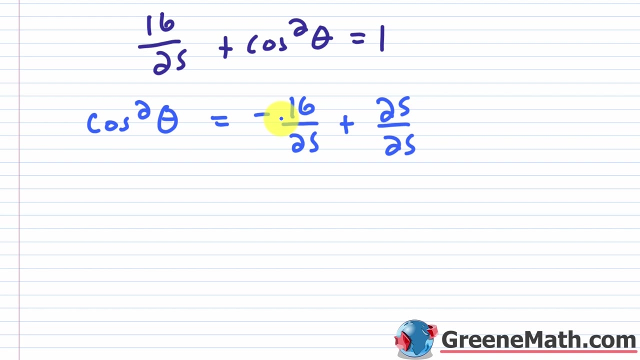 cosine squared theta is equal to. this will be negative: 16 over 25, and then plus 1,. okay, So let's come over here. I know that I need a common denominator now, right, So you can just erase this right now. just put 25 over 25.. So 25 minus 16 is 9.. So I'm going to say cosine squared theta is: 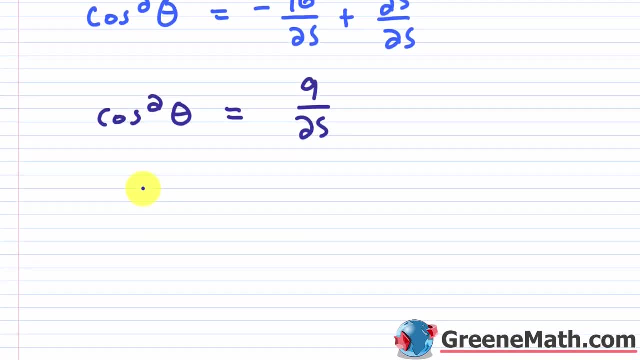 equal to 9 over 25.. So this is where a lot of students struggle. I'm going to put: the cosine of theta is equal to plus or minus the square root of 9 over 25.. Now, which sine should I choose? 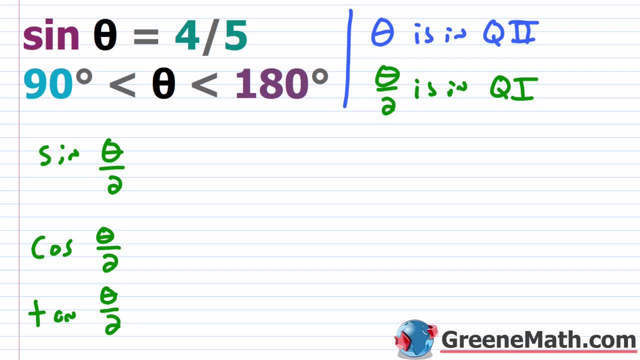 Let's go back up and let's remember that we're working with theta for right now, not theta over 2, okay. So this is where people get confused. They make a sine mistake. So it's theta. Theta is in quadrant 2, okay, If I'm in quadrant 2, cosine is negative. 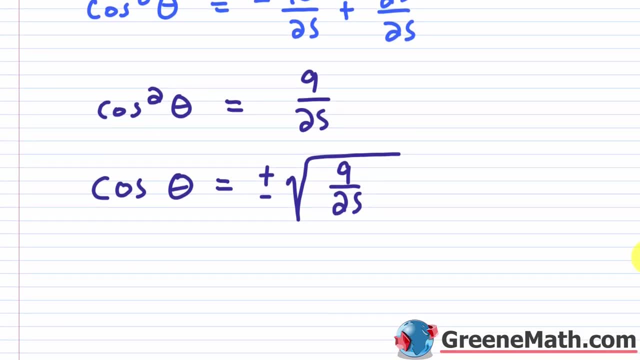 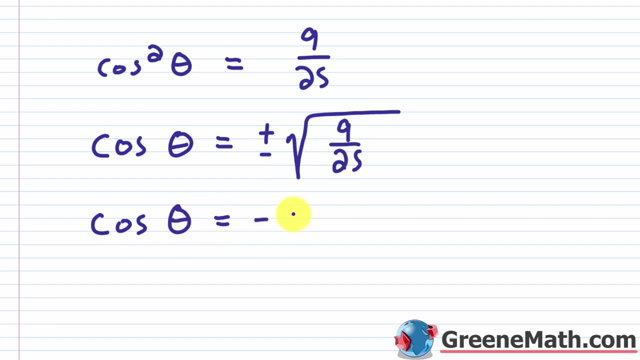 Okay, So that means that in this particular case I want to choose the negative square root. okay, So I want to say the cosine of theta is equal to the negative of the square root of 9 over 25.. So the cosine of theta here is equal to negative 3 over 5, or you could say negative 3. 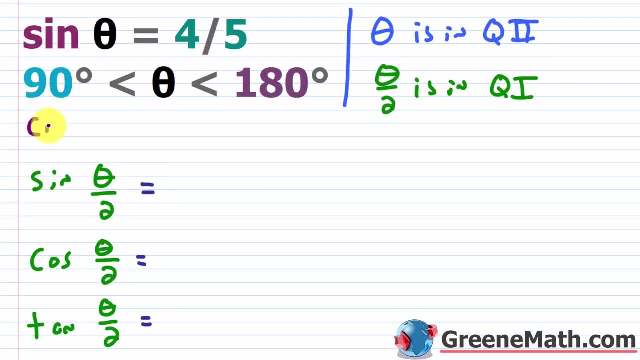 fifths. So let's go back up. So let me write this in here: The cosine of theta is going to be equal to negative 3 fifths. okay, So now we have that And I want to find the sine of theta over 2, the cosine of theta over 2, and the tangent of theta. 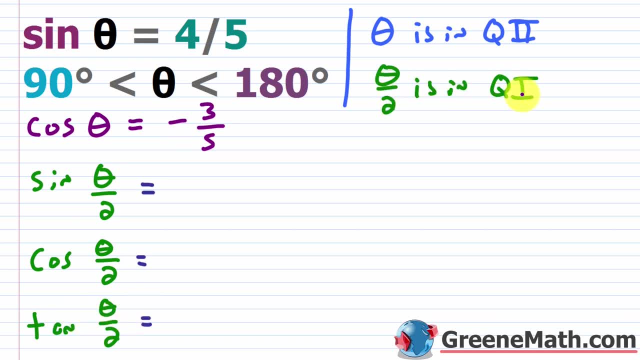 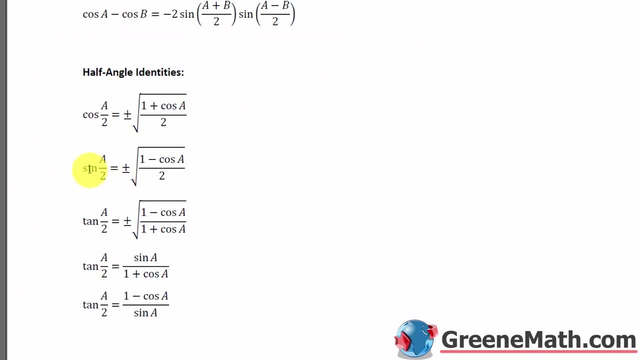 over 2.. Again, we know that theta over 2 is in quadrant 1.. So all of these guys, if there's a square root involved, you want the principal square root, okay? So if I go back to my little sheet, we have the sine: of a over 2 is equal to. again, we just want the principal 1, the square. 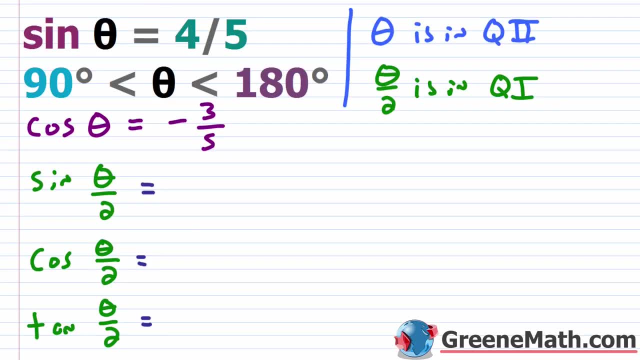 root of 1 minus the cosine of a over 2.. So let me first write this out. So we would have the principal square root of 1 minus the cosine of. in this case, this is your a right. You've got to substitute this. This is theta. this will be. 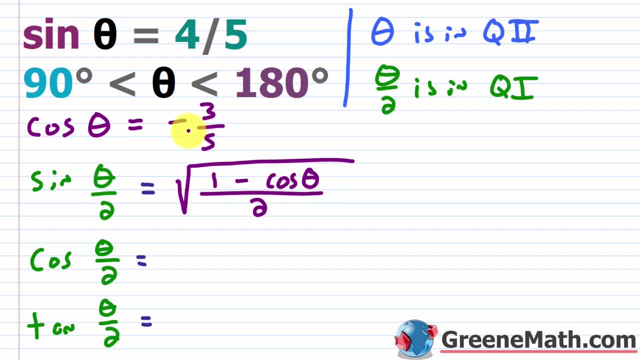 theta here and then this will be over 2, okay, So cosine of theta, we know, is negative 3 fifths, so I'm just going to plug that in. So minus a negative is plus a positive, so I'm going to put. 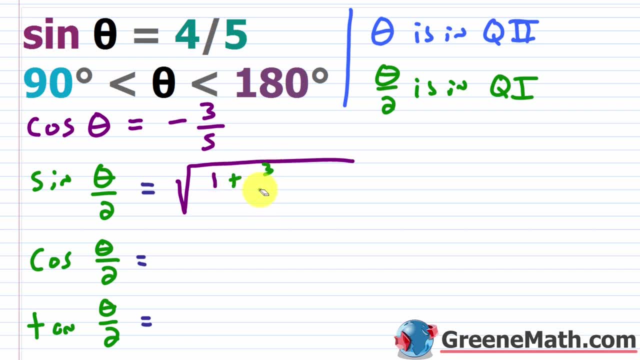 plus 3 fifths. Now how you go about doing this. let me make this better. so 3 fifths like this. How you go about simplifying this is up to you. Of course, you could write 1 as 5 over 5,. 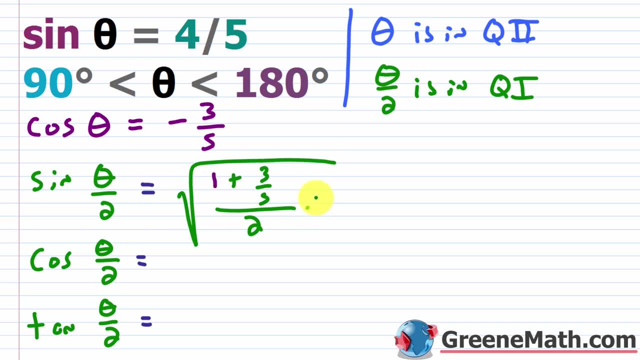 and then basically add your fractions, or you could multiply this here over 10.. It's whatever you want to do, whatever's quicker, Let's just do it this way. So I'm going to say 10 times 1 is 10, okay. And then 10 divided by 5 is 2,, 2 times 3 is 6, so 10 basically, plus 6. 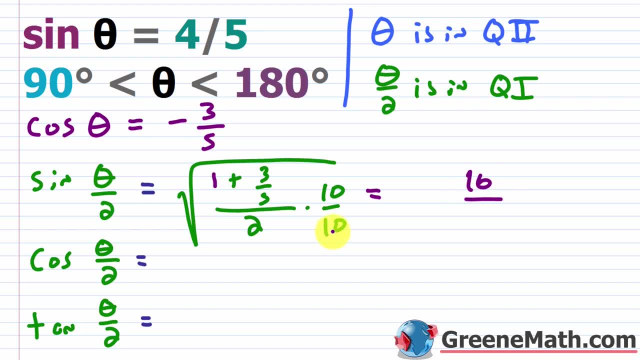 would be 16.. So let's say this is 16 over 10 times 2 is 20, okay, So I'd have the square root of this guy. Let me kind of slide this down a little bit, kind of working with some narrow space here. So 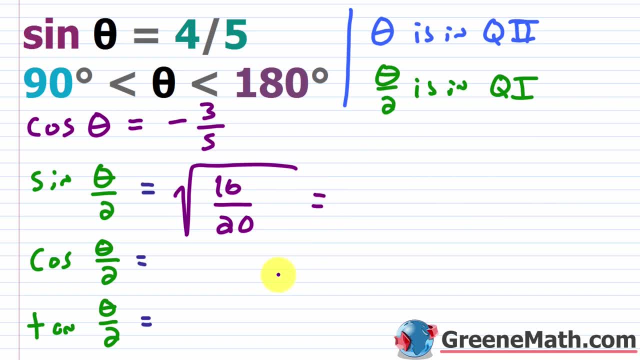 let's come down here and let's put this as equal to: of course, 16 and 20 are both divisible by 4.. So let's put this as equal to. of course, 16 and 20 are both divisible by 4.. So let's put this as: 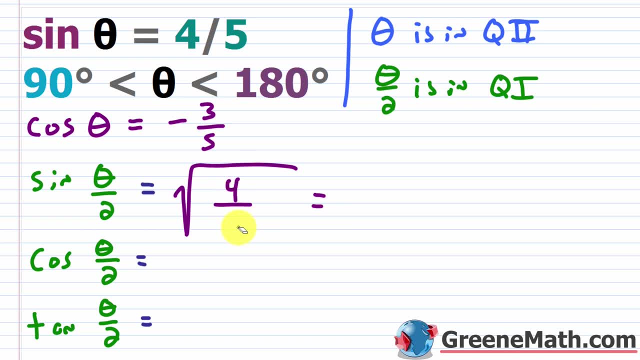 equal to, of course, 16 and 20 are both divisible by 4.. So, divide 16 by 4, you get 4.. Divide 20 by 4, you get 5, right, So what is the square root of 4? fifths, Well, the square root of 4 is 2,. 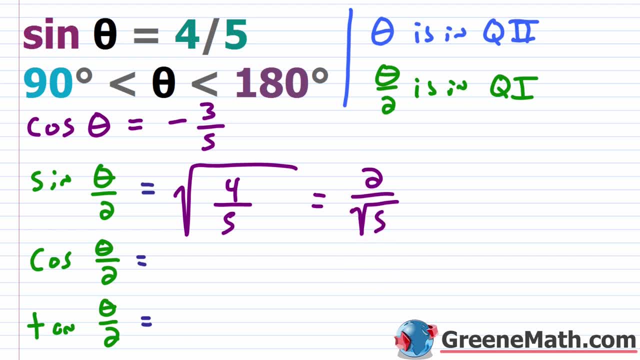 and then over the square root of 5.. Now I need to rationalize the denominator, so I'm going to multiply this by the square root of 5 over the square root of 5., And so this gives me 2 times the square root of 5 over 5, okay, So all that just to get this. 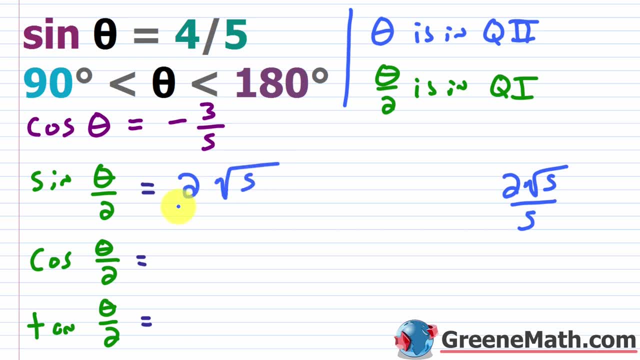 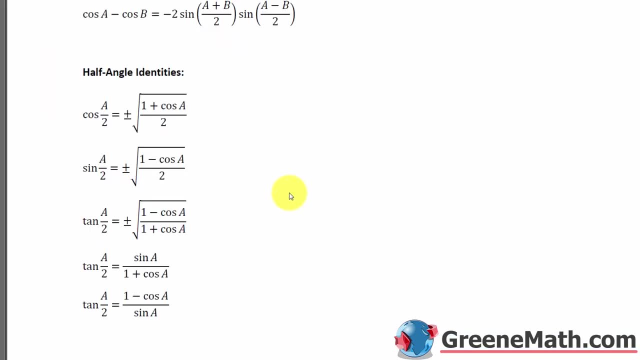 answer here of 2 times the square root of 5 over 5,. okay, Now for the cosine of theta over 2, we have a similar formula. We come back here Again. we're using the principal square root, It's 1 plus the cosine of, in this case it's theta. 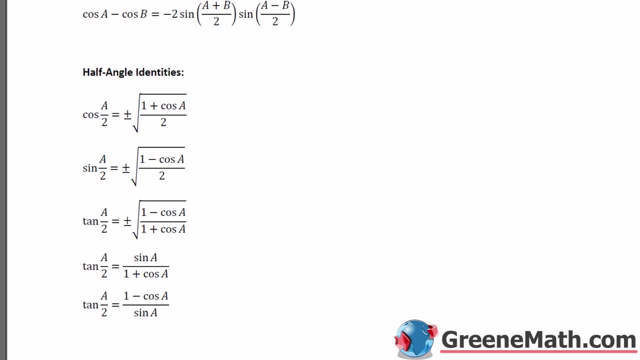 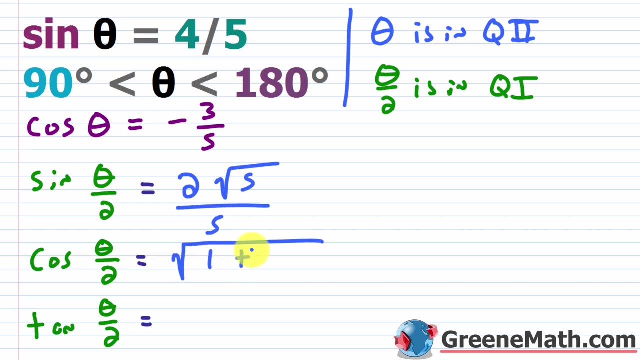 Here it's a, but in our case it's theta over 2.. So let's come back and say this would be what The square root of you have the 1 plus. what's the cosine of theta? Well, it's negative 3 fifths. 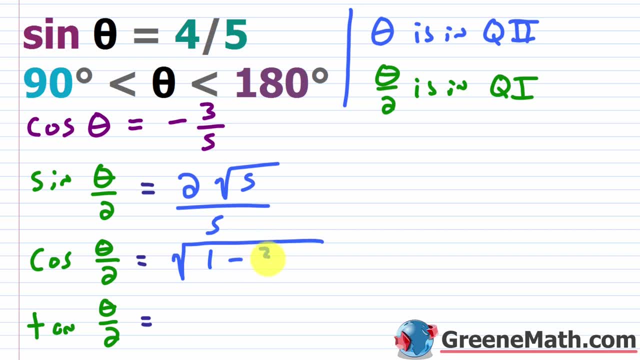 So in this case you don't have the minus and negative, It's straight up minus 3 fifths and then this is over 2,. okay, Let me make this a little bit better and make this longer, like this: Let's come down here. So let's. 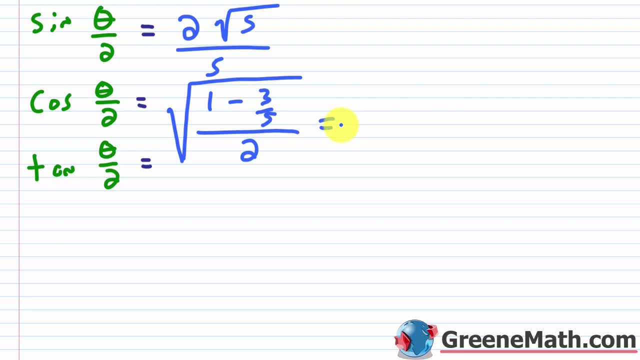 say 1 minus 3 fifths. Let's do this an alternative way. Let's just say this is 5 fifths. okay, So 5 minus 3 would be 2.. So basically you would have the square root of you would have 2 fifths. If 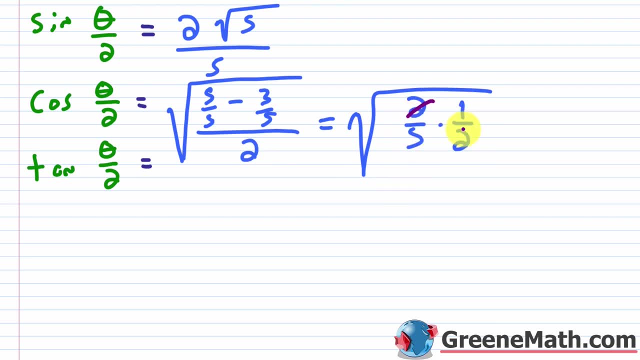 you're dividing by 2, you can just multiply by half, So what you'd have here is the 2s cancel, and so you'd have the square root of 1 fifths. So let's erase all of this and put 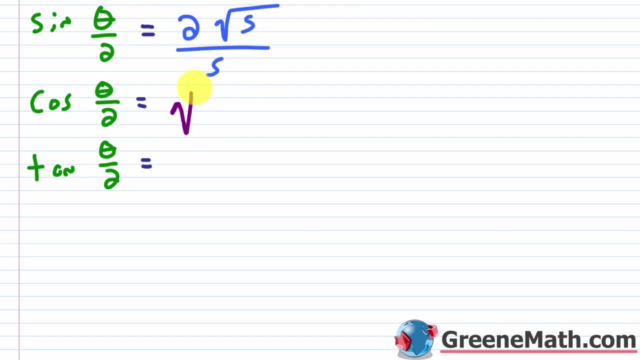 the square root- and I made that terribly so- the square root of 1. fifth, and of course, the square root of 1 is 1, so 1 over the square root of 5.. You need to rationalize the denominator. 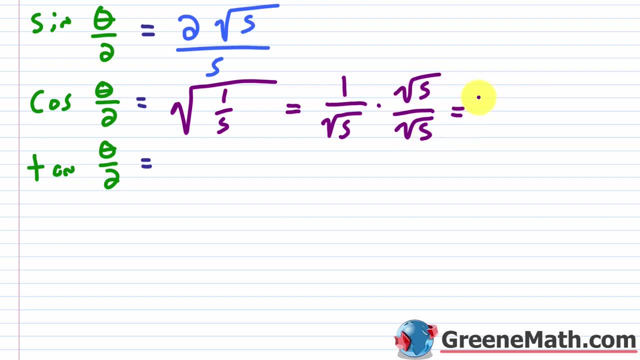 so this is times the square root of 5 over the square root of 5, and so this becomes the square root of 5 over 5,. okay, Let's erase all this and let's slide this all the way down. okay, So this: 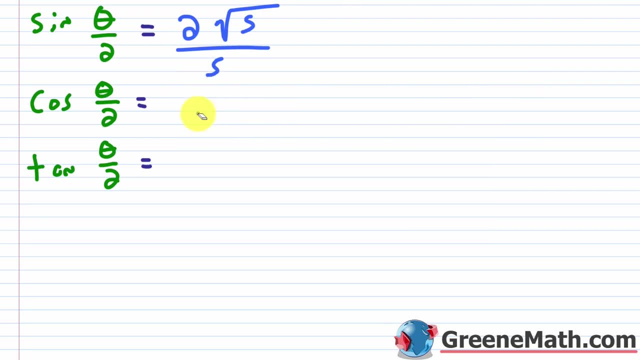 is going to be right there. So square root of 5 over 5, and that's probably too tight. So square root of 5 over 5,. okay, So for the square root of 1, you're going to have the square root of 1,. 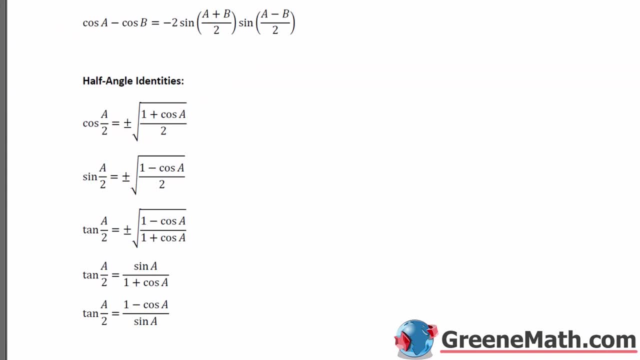 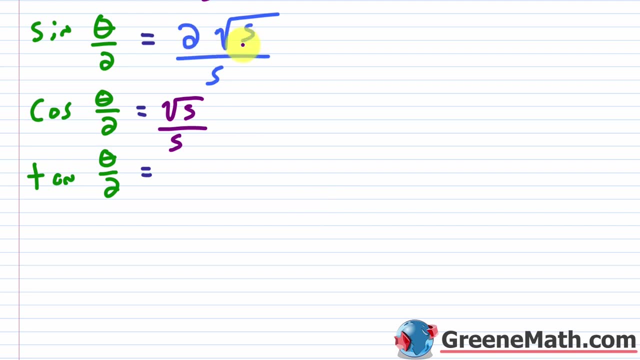 the tangent of theta over 2.. Again, you can come back here and use one of these guys, but again, remember, you can just use your definition of the tangent, okay, So I can just divide this guy by this guy. so I can basically say 2 times the square root of 5 over 5.. If I'm dividing with 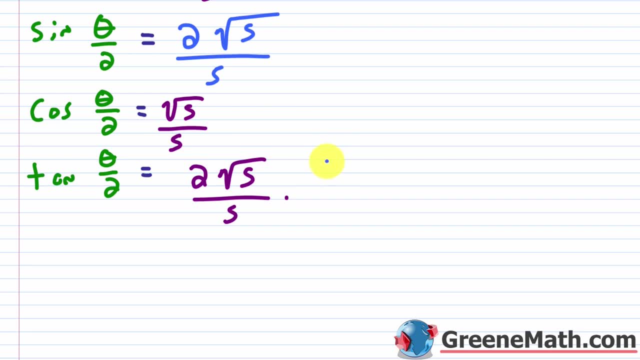 fractions. I just multiply by the reciprocal. So I'm going to flip this and I'm basically going to have 5 over the square root of 5, and so we see that this would cancel. okay, This would cancel and I just get 2, okay, So the tangent here is going to be 2.. 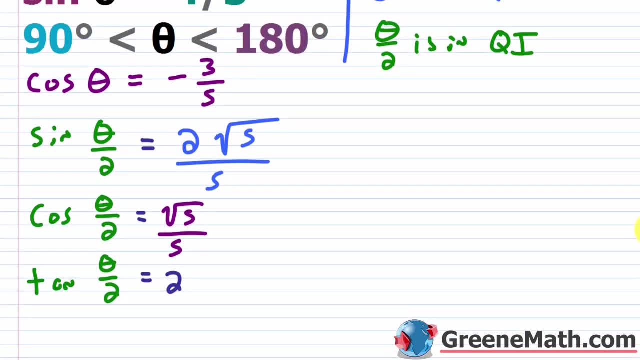 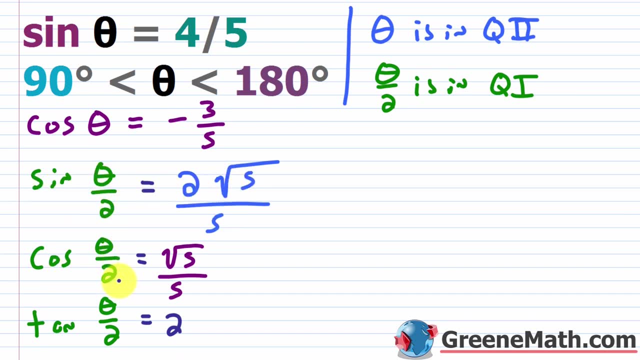 So now we've found all of the guys that we were looking for. So if we're looking for the sine of theta over 2, it's 2 times square root of 5 over 5.. The cosine of theta over 2 is square root of 5. 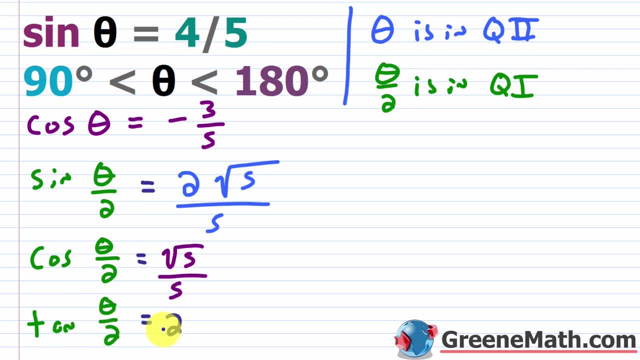 over 5, and the tangent of theta over 2 is just going to be 2, okay, So again, if you wanted to find the other ones, you could flip this guy right here in order to find your cosecant of theta over. 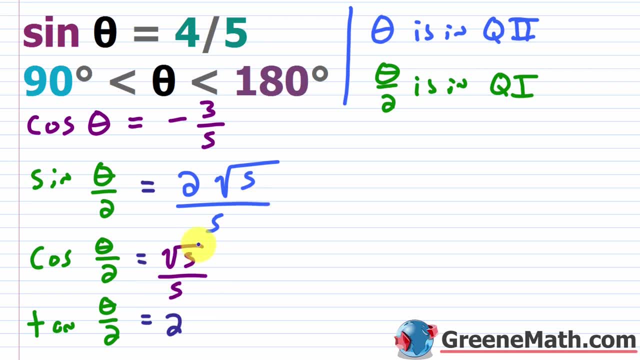 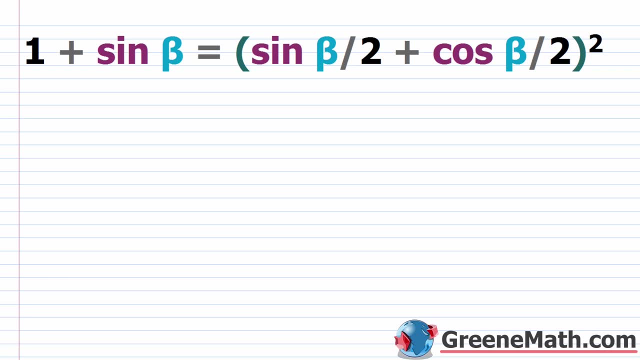 2, flip this guy right here in order to find your secant of theta over 2, and flip this guy right here to find your cotangent. Alright, let's look at one more problem here, and this just involves verifying an identity. 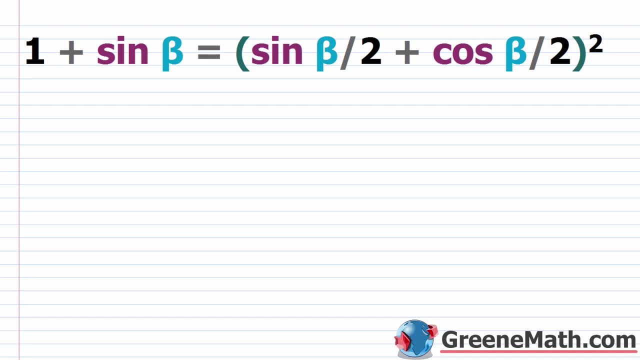 It's just important to get a lot of practice with this, not only for calculus, but because in this section in trigonometry, it just keeps coming up over and over and over again and there's no general set of rules to follow for this. It's all just practice, right? So? 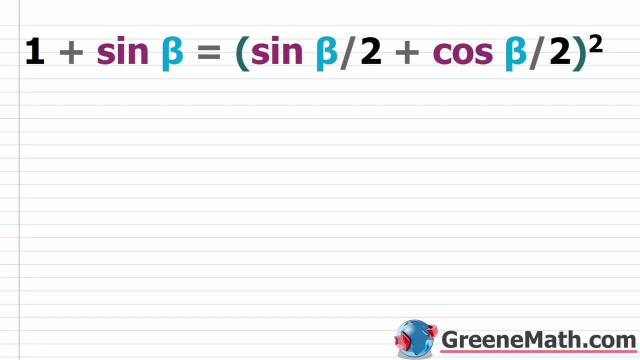 manipulating things, trying to make sure it works out, and then just keep going. As long as you're making proper algebraic substitutions, you will eventually get where you want to go. okay, If I look at this, I have 1 plus the sine of beta is equal to this quantity, sine of. 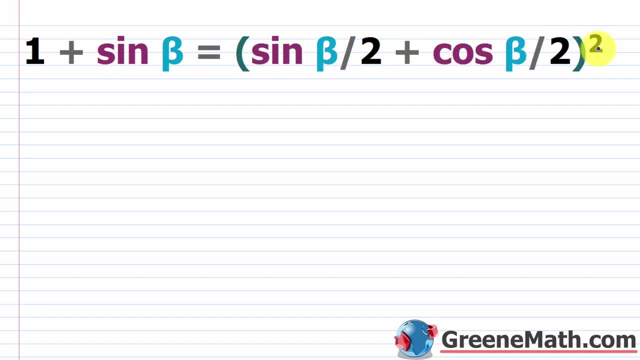 beta over 2 plus cosine of beta over 2 squared okay. So obviously the left side here is much simpler, so I'm just going to work on the right side. Normally, you put your equal sign in line here, but I'm going to have to move this all the way over here just because I'm going to run out. 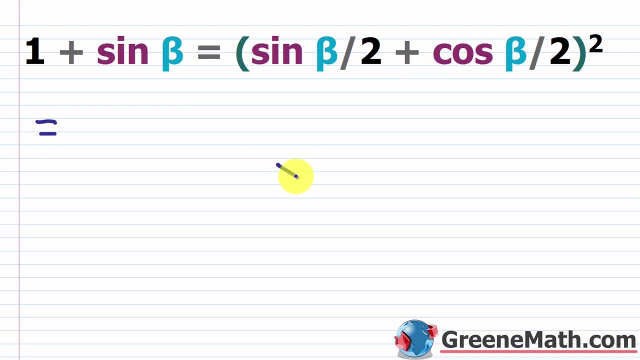 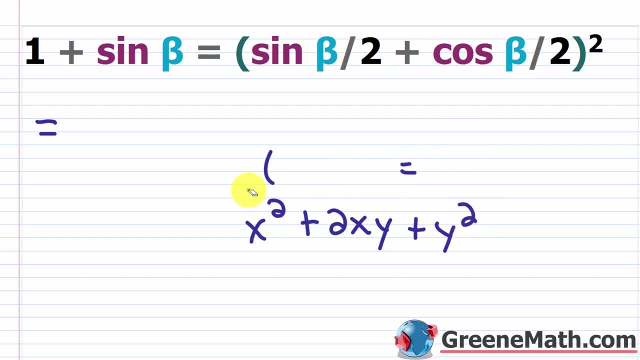 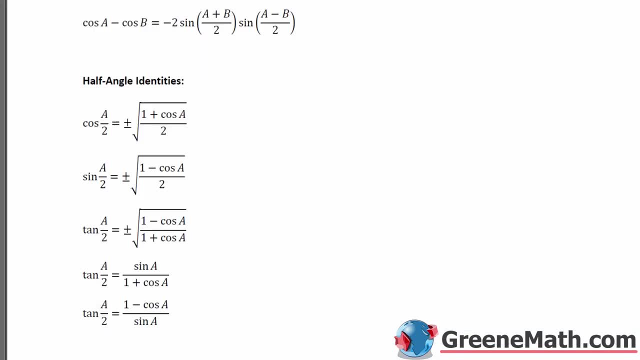 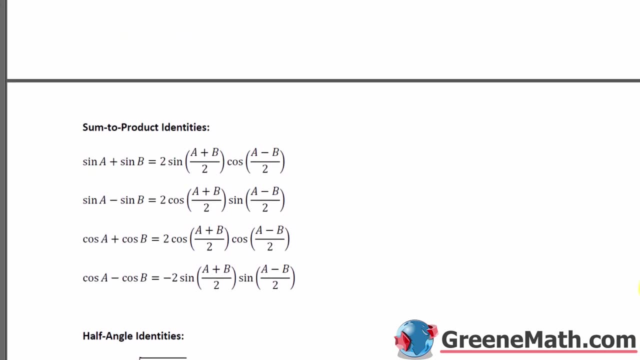 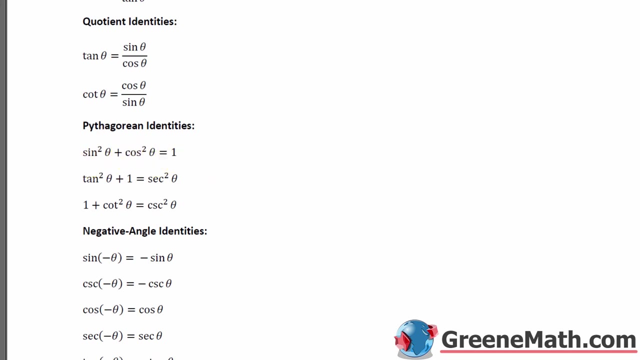 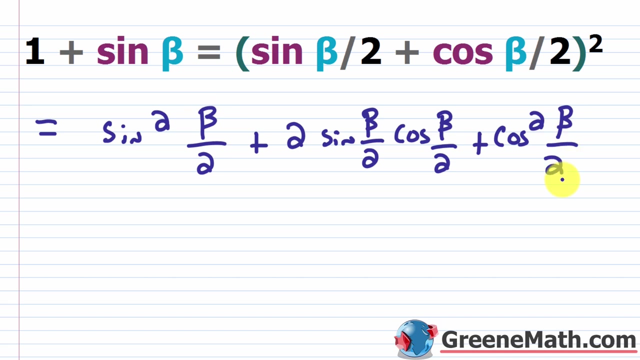 Here you want to think about. if I look at this guy, what do I have here that I can maybe do something with? So nothing really. with the half angle identities You actually have to go all the way back up to the Pythagorean identities. Remember, we used this earlier. the sine squared theta plus the cosine squared theta equals one. Okay. so if we think about this, we have sine squared of beta over two, so there's just some angle plus cosine squared of that same angle, beta over two. So this plus this would be one. Okay. so I can just basically say that. 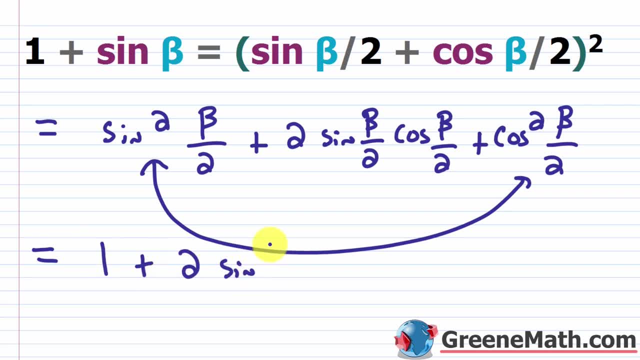 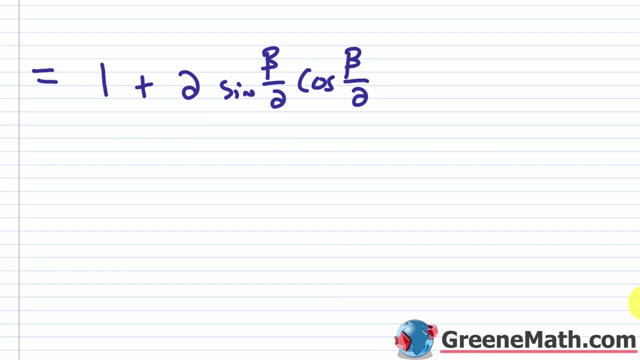 that's one plus your two times sine of beta over two, times the cosine of beta over two. let me get rid of this marking here because I kind of in the way, And from here you're really thinking about now, your double angle identities from the last section. Okay, remember what you're trying to get. 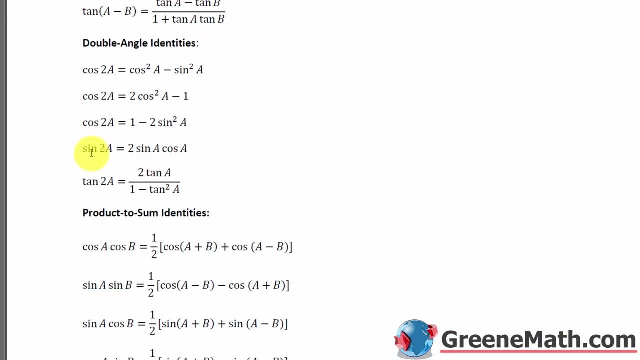 to. If you look at this, you have one plus the sine of beta. So for this guy right here we have the sine of two. a is equal to two times the sine of a times the cosine of a. Okay, so this is what. 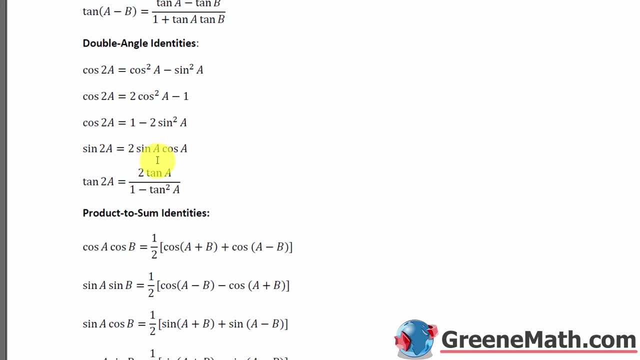 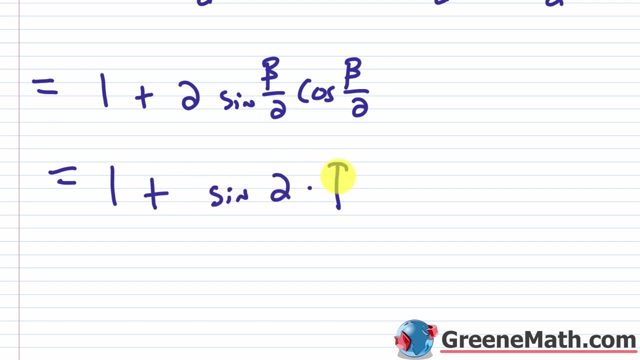 I have here, right, I have two times the sine of beta over two, times the cosine of beta over two. So I'm going to go and write it like this: sine of two times beta over two. Okay, so I want to put this as one plus, we'll say the sine of two times beta over two. the twos are going to cancel, And 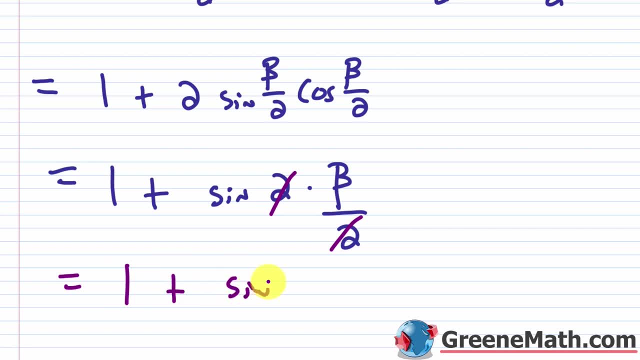 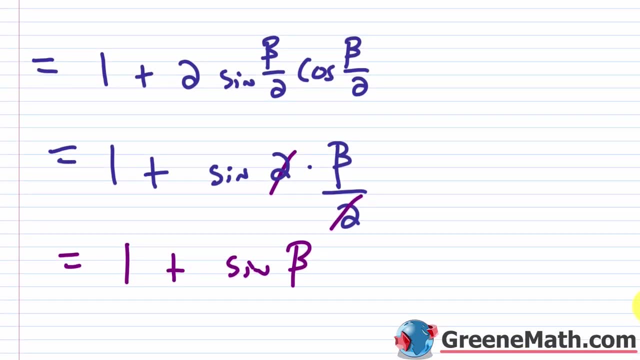 look at what I have. I have one plus the sine of beta. Okay, if I go back up I'm looking for one plus the sine of beta. So bam, we got. and I know these things are kind of hard. I've obviously 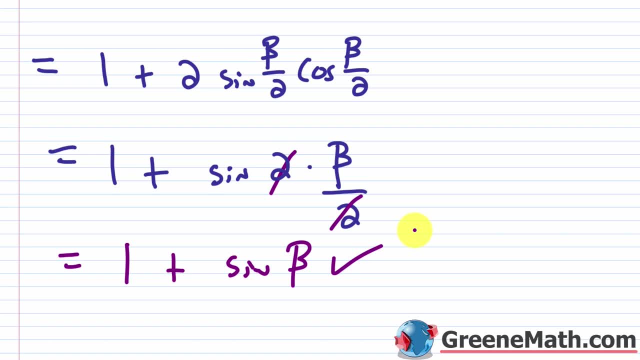 already worked the problem, So I know what to do. But when you're working with these, don't get frustrated Again. you can always try to put things in terms of sine or cosine before many factoring, before many squaring, And just get as much practice with these as you can, Because when you get to the 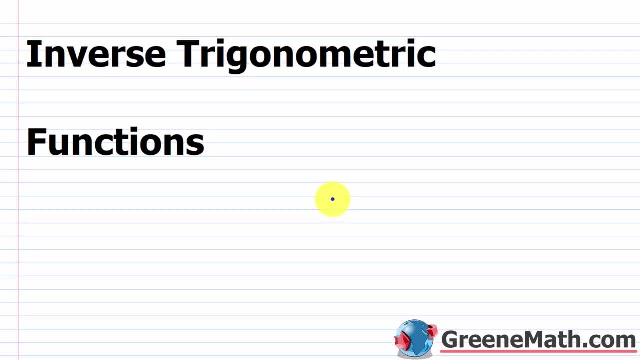 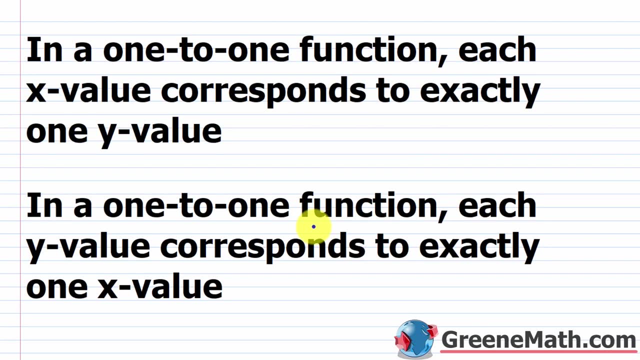 test. you have to get them done in a reasonable amount of time. In this lesson we want to talk about inverse trigonometric functions. Alright, so before we get into the inverse trigonometric functions, I want to recap some things that we talked about earlier in the course. 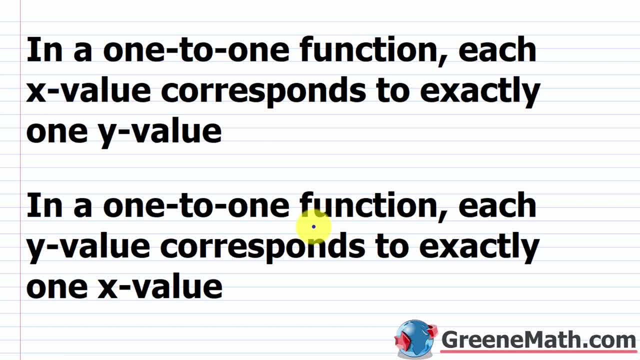 it's gonna be really important that you understand this information in order to fully understand this lesson. So, first and foremost, we discussed the idea of a one to one function. So in a one to one function, each x value corresponds to exactly one y value, And additionally, you could say in a one 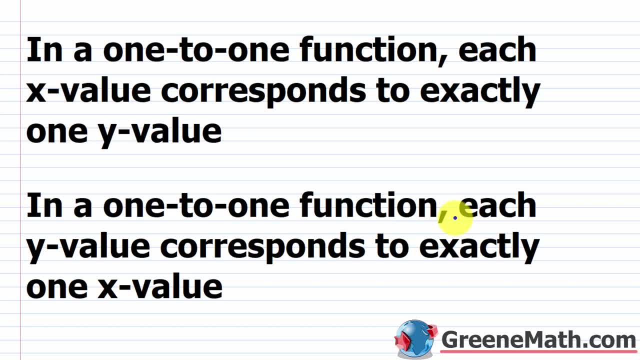 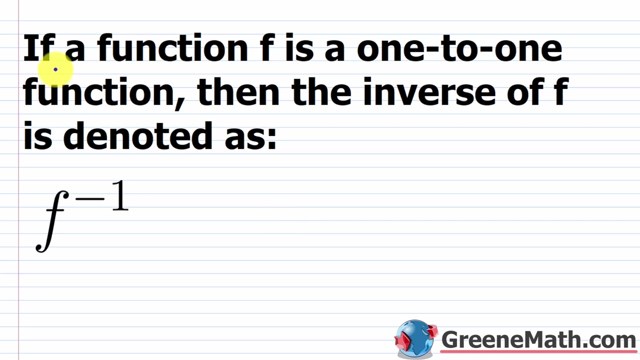 to one function, each y value corresponds to exactly one x value. So often you'll hear, for example, if you have a one to one function, you can verify that using something called the horizontal line test. So for the horizontal line test, if you have the graph of a one to one function, no horizontal line will impact that graph in more than one location. So a common source of confusion when you work with inverses would be the notation that's involved. So I have here: if a function, f, is a one to one function, then the inverse of f is denoted, as here. this is f inverse. So again, this is the 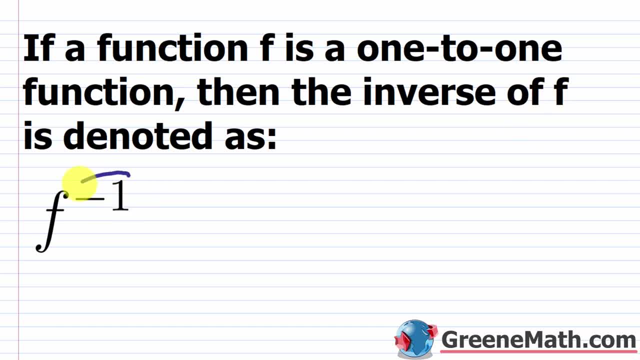 inverse of my function f. Now, this, right here, is what you have to get straight. This is not an exponent of negative one. that is a very common source of confusion. Later on in this lesson, when we get to inverse trigonometric functions, you'll see something like y is equal to the inverse sine of x And that's one way to write it. we have a different way to write and I'll get to that later on, But you need to know that this is not an exponent of negative one. This is telling me. I have the inverse sine of x. Now, provided that your function- let's just call it f- 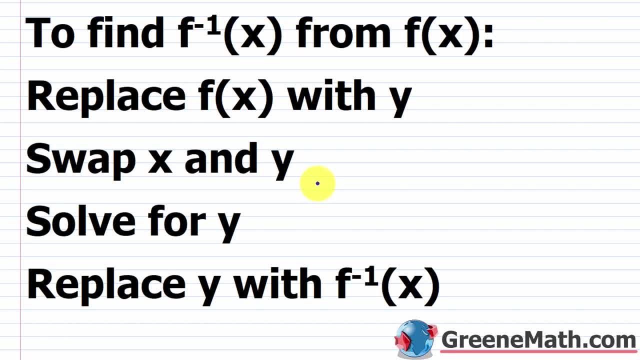 of x. x is a one-to-one function. you're going to be able to find the inverse using this little procedure. so to find the f inverse of x from f of x- again, f of x is a one-to-one function. here we're going to 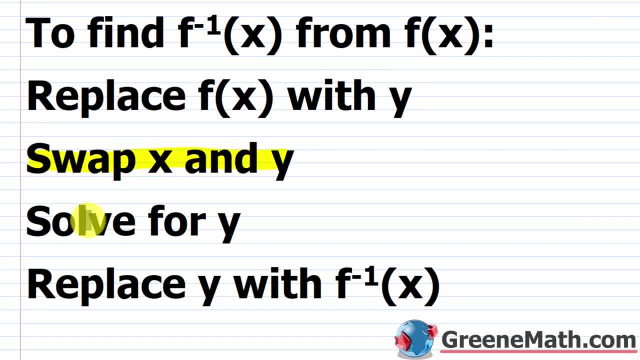 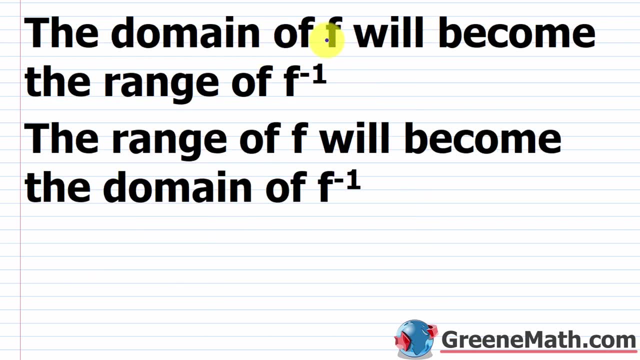 replace f of x with y. we're going to swap x and y, then you're going to solve for y and then, once you've done that, you're going to replace y with f, inverse of x. so this right here, this swapping x and y, this leads to the following: so we have that, the domain of f. so the domain, remember, is the set. 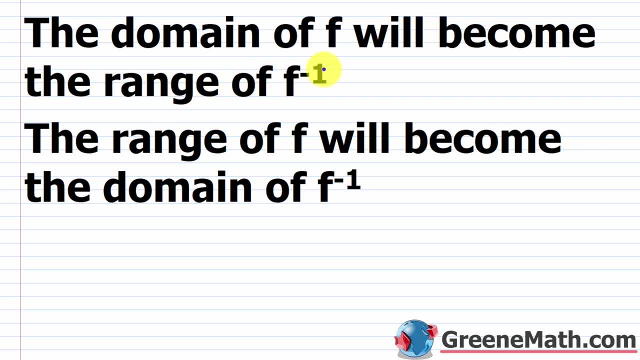 of allowable x values will become the range of f inverse, so the range is the set of allowable y values. so again the x's and the y's were switching places. so that's what's causing this. the domain of f or the x values will become the range of f inverse or the y values, so the x's and 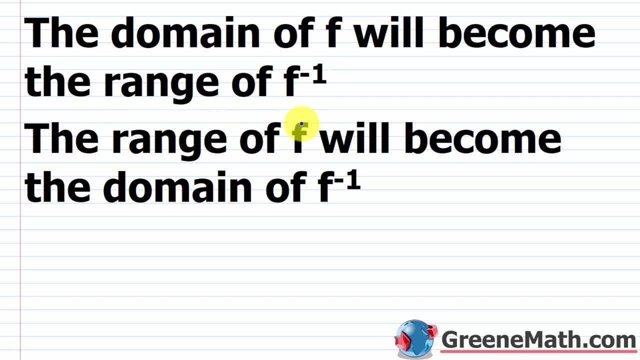 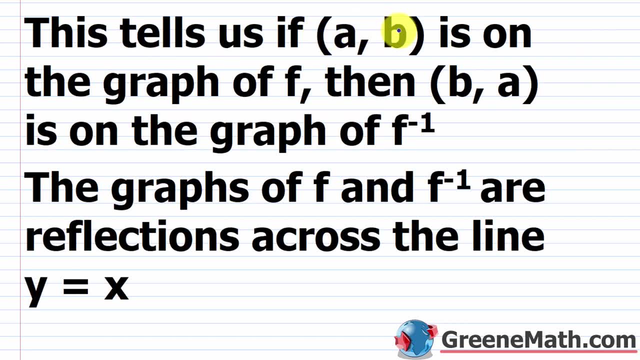 the y's are switching places. similarly, the range of f will become the domain of f inverse. again, the x's and the y's are switching places. so this tells us: if a comma b is on the graph of f, then b comma a is on the graph of f inverse. so notice that these guys switched roles. 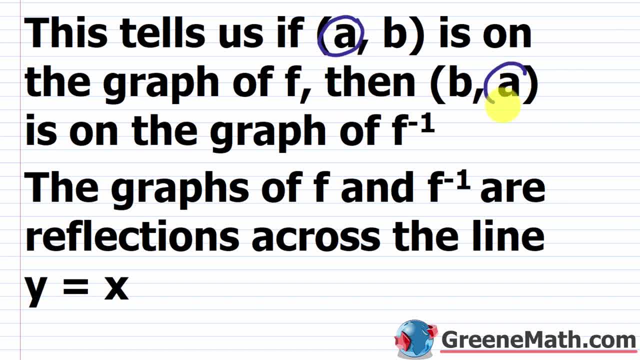 so here, this is your x, and then here it becomes your y, and then here this is your y, and then here it becomes your x. so again, the domain of f becomes the range for f inverse, and the range of f becomes the domain for f inverse. so your x's become. 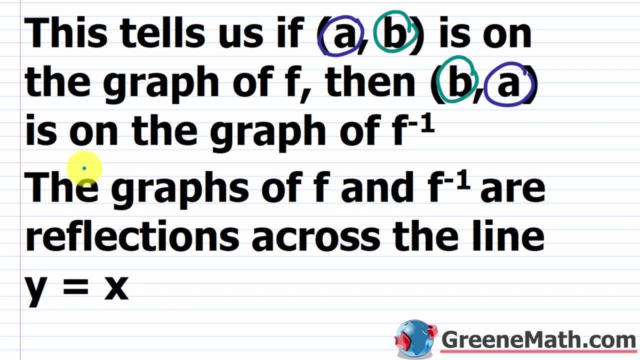 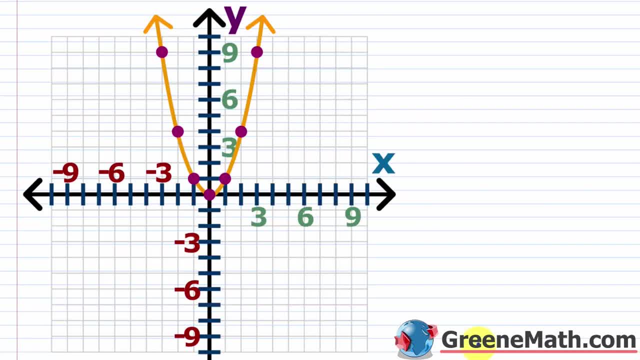 the y's and the y's become the x's very important. and then i have here the graphs of f and f. inverse are reflections across the line y equals x. so there are many cases where we're going to have a function that's not a one-to-one function but we still want to find the inverse. so in that, 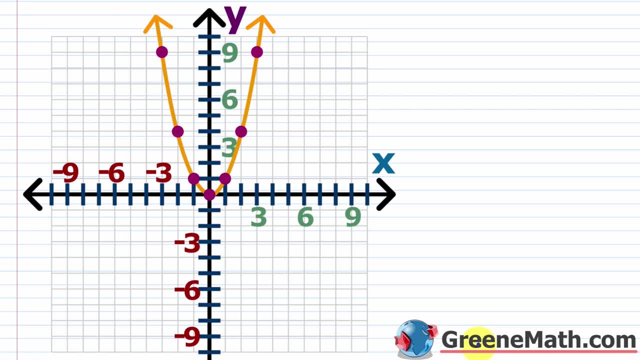 situation. what can we do? well, let's start off with something that we did earlier in the course. we looked at the squaring function. so this graph right here is for f of x is equal to x squared. so clearly, this graph is going to be a one-to-one function, so we're going to have a function that's. 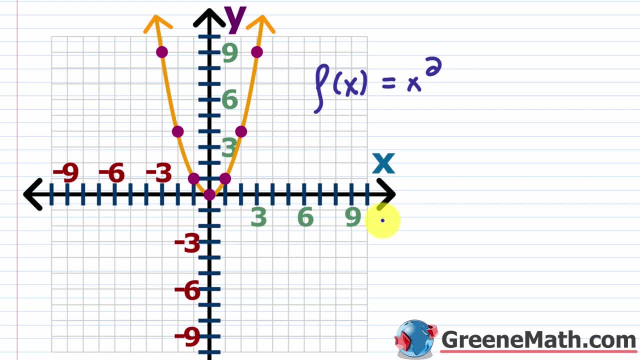 not a one-to-one function. let's just use the horizontal line test real quick to prove that. so this would be: the line y is equal to four. now, if you look at this horizontal line, it is impacting this graph of f of x equals x squared in two locations. so right here and then right here. 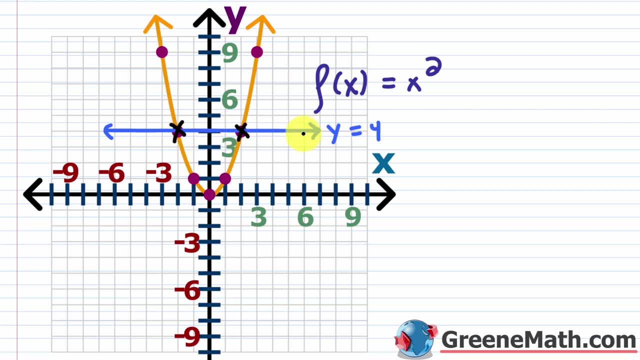 so again, if you have the graph of a one-to-one function, no horizontal line will impact that graph in more than one location. so this right here will not be a one-to-one function. if you look at the graph of a plus or minus function, we're going to have a function that's equal to 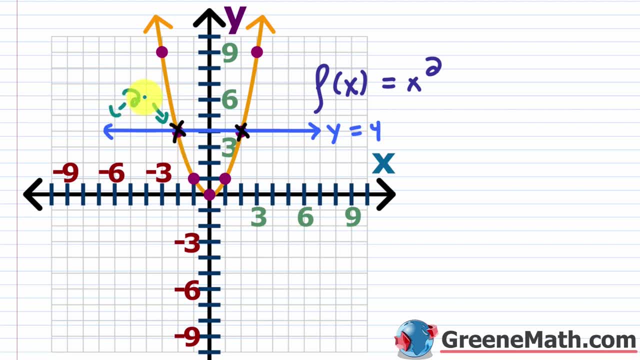 two units to the left and four units up, so this is negative two comma four. if I look at this point right here from the origin, I'm going two units to the right and four units up, so this is going to be two comma four. so the issue is that this y value of four is associated with two different x values. 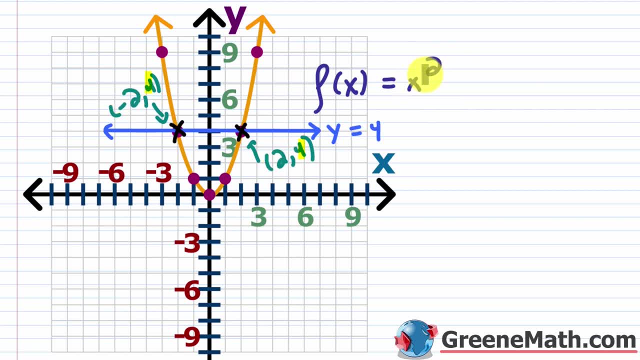 here with negative two and here with positive two, and that's coming from that squaring operation. if I plug in a two for x, two squared is four. if I plug in a negative two for x, negative two squared is also four. So when this happens, what can we do? Well, like we saw earlier in the course, we can impose a. 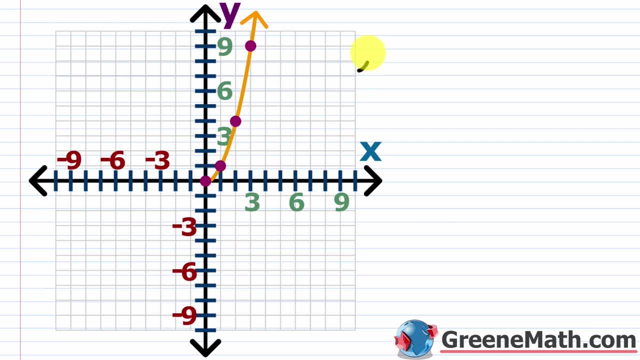 little domain restriction. So for this graph right here we start with f of x equals x squared. So that's the squaring function. But you would notice that it seems like I've cut off anything to the left of zero. So basically we would say that x here is greater than or equal to zero. So this: 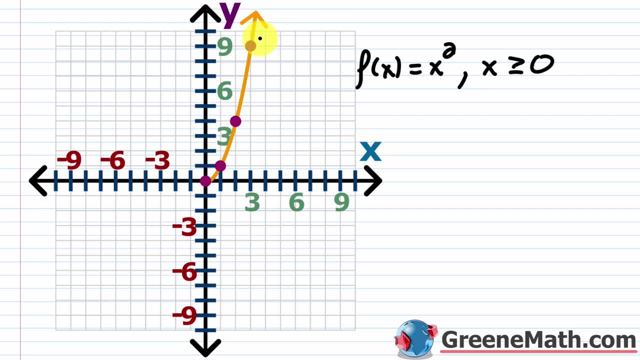 is going to create a one to one function And this is the key. the range is going to be the same. So we're going to see that's going to be important as we get into these trigonometric functions and the inverse trigonometric functions that we create from restricting the domain. So the range here is: 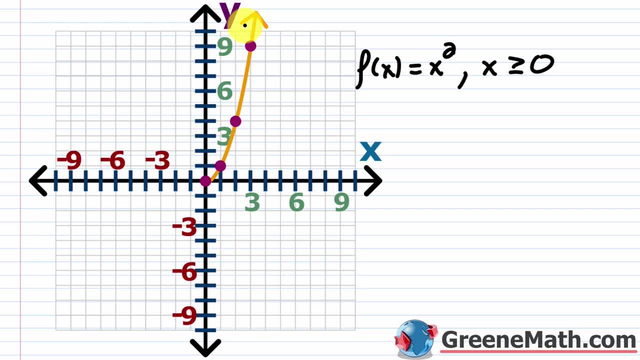 the same. before it was from zero to positive infinity, And now it's still from zero to positive infinity. Now let's just prove that real quick. I'll just put in this same horizontal line here. So again, this is: y is equal to four. And notice that now when I draw this line, it's going: 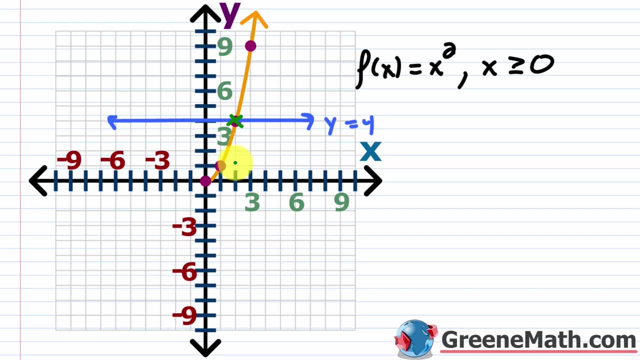 to impact the graph only in one location, And that's true for any horizontal line that you would draw here. So this is now the point two comma four. my point negative two comma four, that was on the other one where I didn't restrict the domain. that's gone because x can't be negative two here. 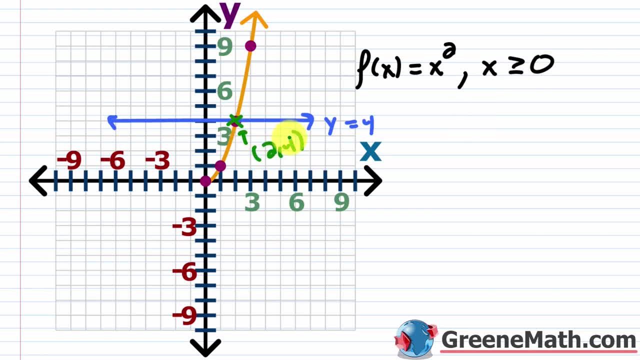 x can only be zero or anything larger, So I only get two comma four. So basically, in the inverse I'm going to have four comma two, right? So two comma four, and then four comma two. So for each x there's one y, And now for each y there's going to be one x, So I'll be able to find an. 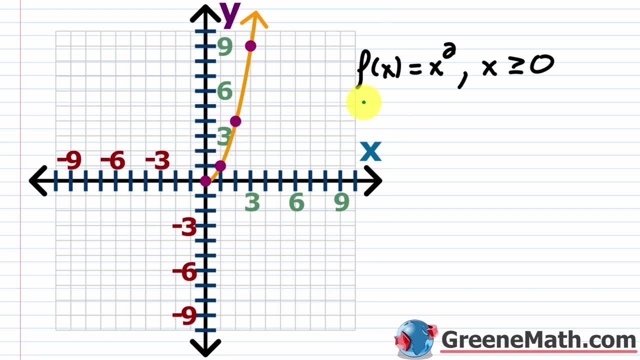 inverse. Okay, so let's just go through that real quick. Hopefully you know how to do this from. if not, let's just go through it once So that later on it'll be easy. So, basically, you start off by replacing f of x with y. So let me write here that we're going to find the inverse And 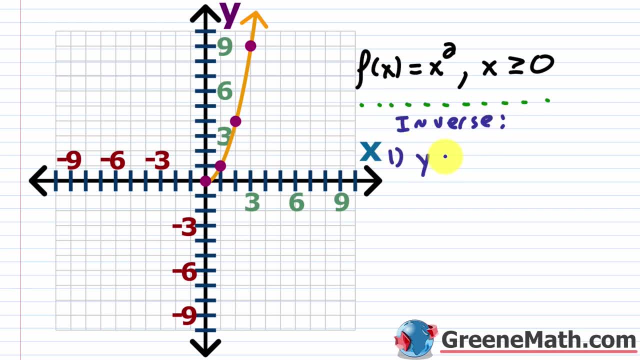 you would start by replacing again f of x with y, So y equals x squared. then the next step is to swap x and y. So we're going to say that we have x is equal to y squared. So this y became x. 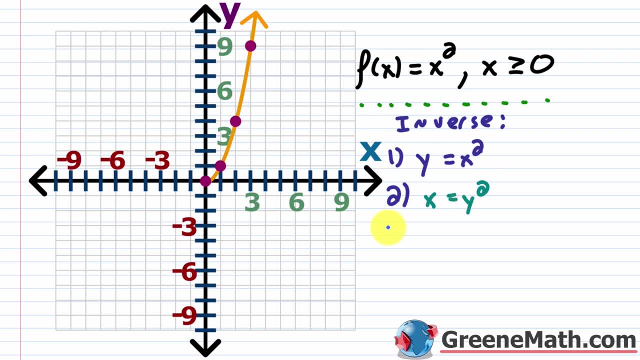 this, x became y. that's all you're doing. Then your next step, you're going to basically solve for y. So first I would write this as y squared equals x, As my personal preference goes. I like what I'm solving for to be on the left, And then I would use the 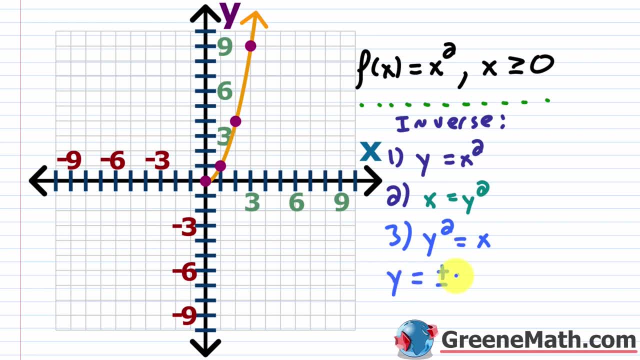 square root property. So you would say that y is equal to, plus or minus, the square root of x. So here's where we have to pause and think. In this function, right here, that's domain restricted- f of x equals x squared. we said that x is greater than or equal to zero. Well, we know that the 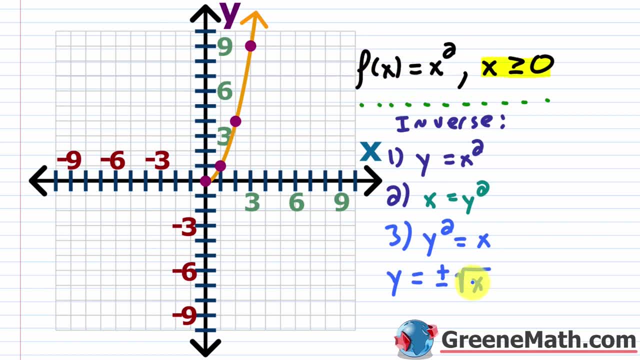 domain from this function right here becomes the range for the inverse. So specifically here I would say that y is greater than or equal to zero. So I don't need this plus or minus here because I can't have the negative of the square root of x, because I'm specifically saying that 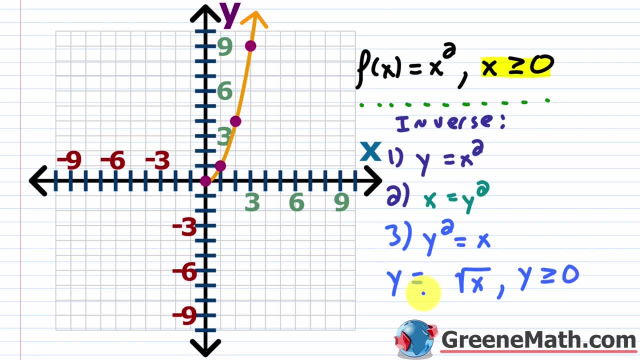 y is greater than or equal to zero. So I'm going to get rid of this plus or minus and say that y is going to be the principal square root of x. So let me replace this with: y is equal to the principal square root of x, And I'll get rid of this. And then step four is just to replace your. 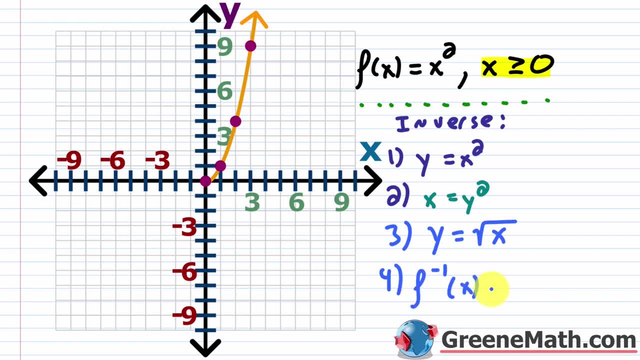 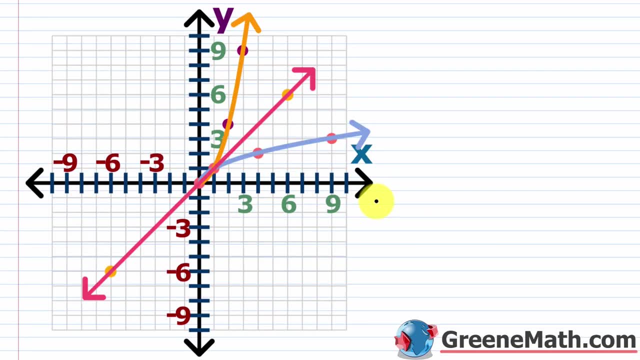 y with your f inverse of x, And so this is equal to x squared. So I'm going to get rid of this to the square root of x. All right, so before we move on, it might be helpful to look at this graphically. This is especially useful when you're trying to figure out if you've got the right. 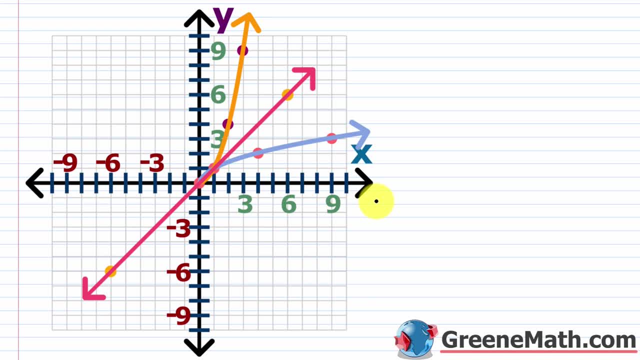 inverse. Remember that a function and its inverse are going to be reflections across the line. y equals x, So you can always look at this graphically and see that. So this graph right here for this guy in orange, this is our f of x equals x squared, where we said that x is greater. 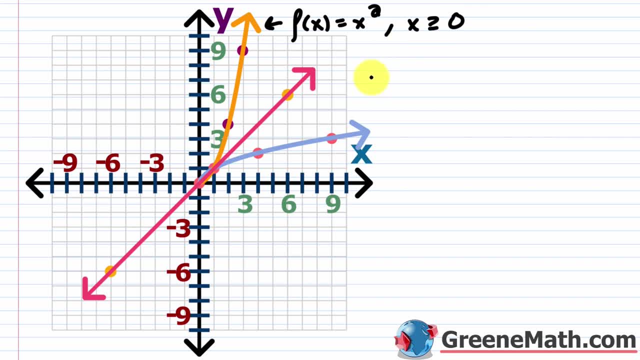 than or equal to zero. If you're going to do this on Desmos, you want to do this as f of x equals x squared, And then you're going to open up some brackets and you're going to put in your restriction- So x is greater than or equal to zero, and then just close those And it'll give. 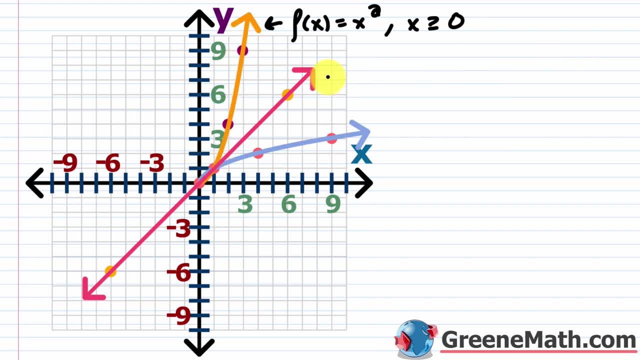 you this graph here in orange: Okay then the graph in red- this is just the line y- is equal to x, So you can put f of x equals x, whatever you want to do. And the graph in blue: this is our inverse. So f. inverse of x is the square root of x. I'm just going to put this as g of x, So f. 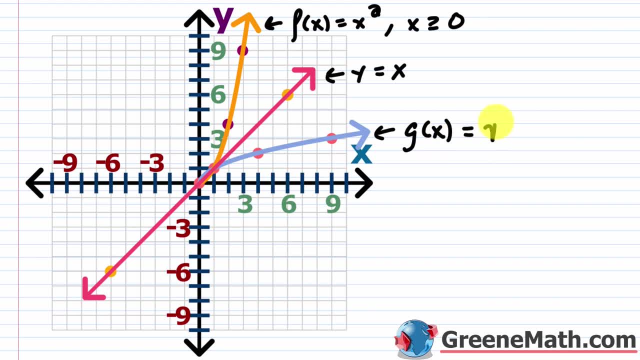 of x and g of x. those are going to be inverses And this is equal to just the square root of x. Now what you can do is look at a few points and just prove a few things. So, first off, let's just 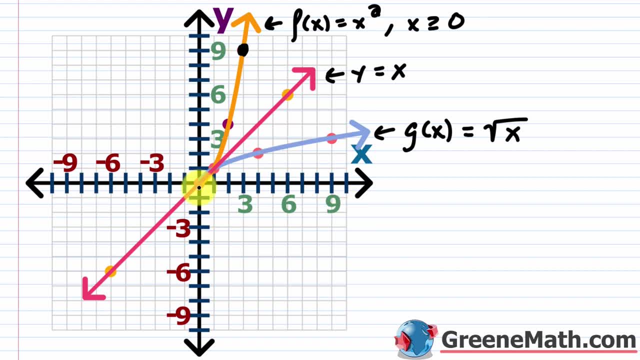 start with this point right here. So this point right here I'm going three units to the right and nine units up from the origin. So this is going to be the point. let me arrow to this. So this would be three comma nine. Now again, if I reflect this across the line, y equals x. 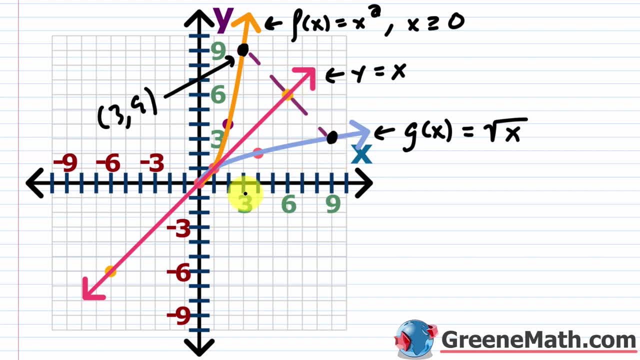 I'm going to get this point right here. So this point right here would be nine comma three. So this point right here, which was three, is going to become the y value here, And the y value here, which is nine, is going to become the x value here. So the x's and the y's are switched. 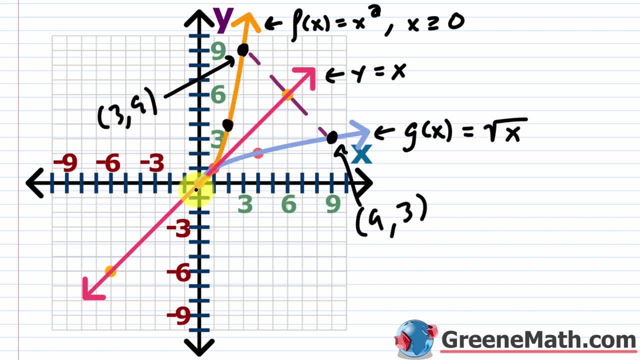 then let's just do one more. So this point right here, if you look at it, is going to be two comma four. So this point right here is two comma four. And then, if you look at again, reflecting across the line y equals x, you're going to get this point right here And now, instead of two comma four. 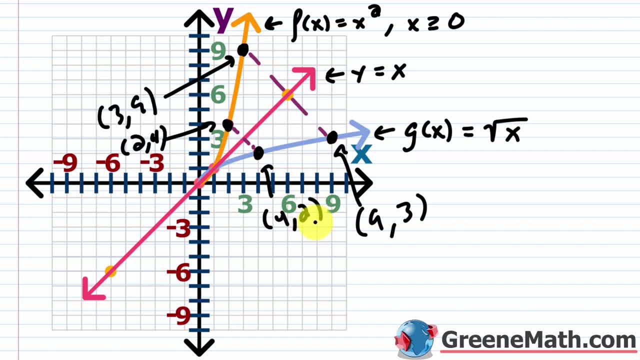 you're going to get four comma two. This is always something you can use if you're trying to figure out if you got the right inverse. it's very helpful to graph your function, graph your inverse and graph the line y equals x And 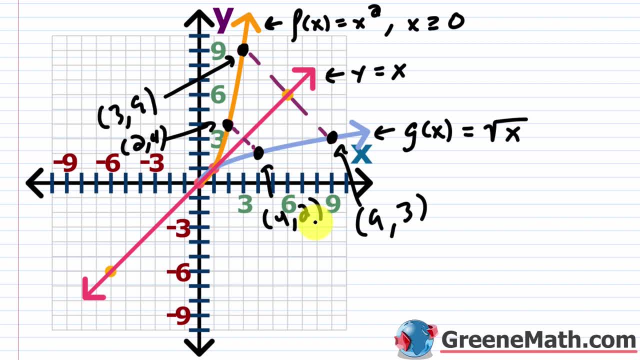 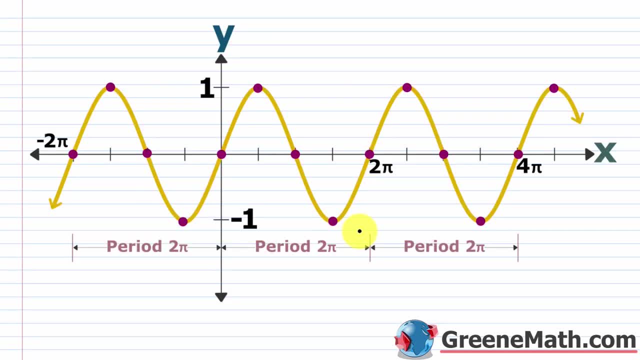 just look at: if your function and the inverse are reflections across the line y equals x, then you know you got the right one. All right, now let's move on and talk about how to find the inverse trigonometric functions. we're going to start off with how to find the inverse sine. 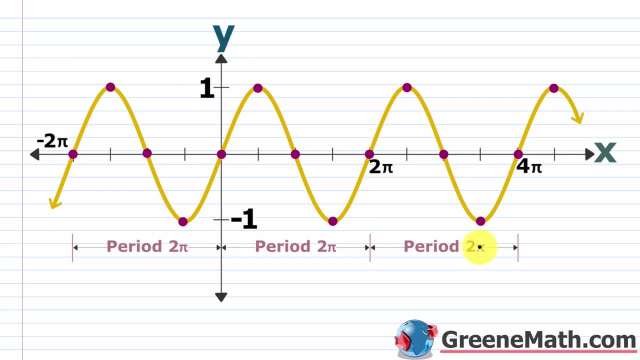 function. And so to do that we're going to begin with our graph of f, of x equals the sine of x, of x is equal, to say y is equal to the sine of x. So we study this graph earlier in the course. 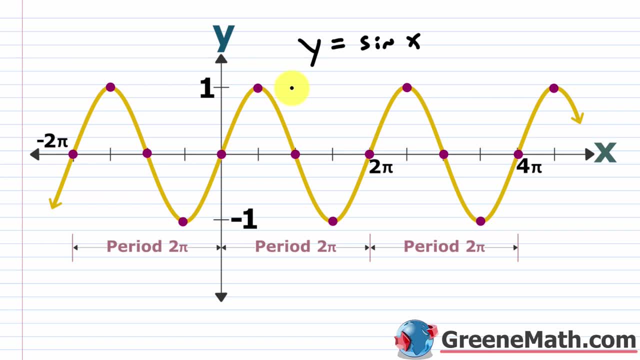 At this point you should know that the domain is a set of real numbers and the range is from negative one to positive one. So let me write this out. So the domain is going to be the set of real numbers, So from negative infinity to positive infinity, So that 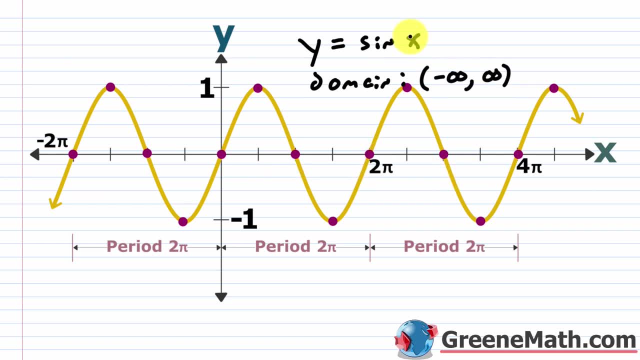 means I can plug in any real number I want for x here. So a negative, zero, positive as long as it's. I'm good to go Then in terms of the range. so in terms of the range we can see, that's from. 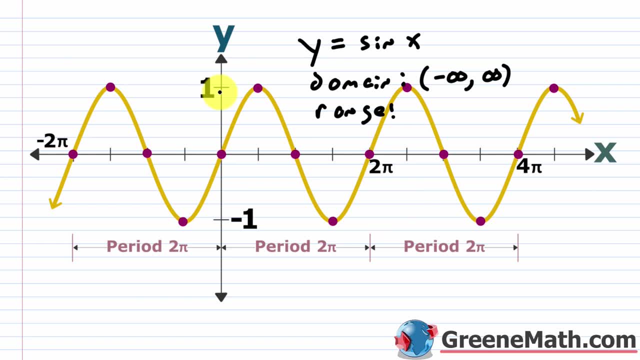 negative one to positive one, And you should know that from the unit circle. So let's go ahead and put: from negative one to positive one. Clearly, this guy is not the graph of a one to one function. If I draw a little horizontal line like this, well, you can see that I'm going to hit here. 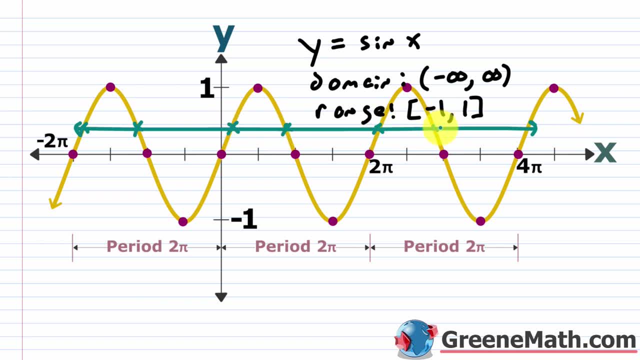 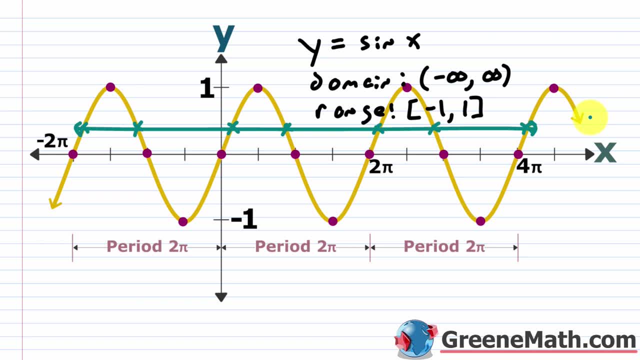 line test. So what can we do when we encounter this situation Again? just like with the squaring function, we restricted the domain such that we have the same range. So let me actually erase this and show you what we're going to do. we're going to take a piece of this graph, So we're going to 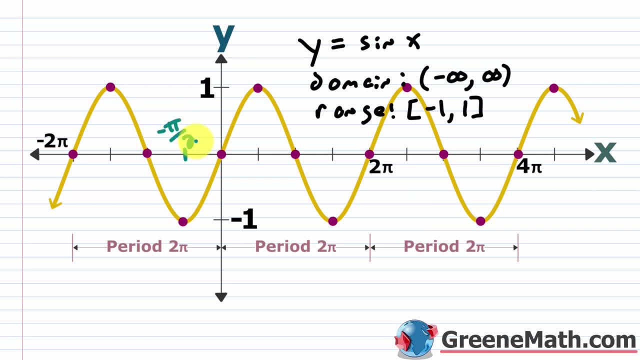 go from right here- this is negative pi over two- to right here- this is pi over two. let me write that A little bit more neatly. So again, this is negative pi over two here. So you're going to take right here to right here, So just a piece of that graph right there, And now it's going to 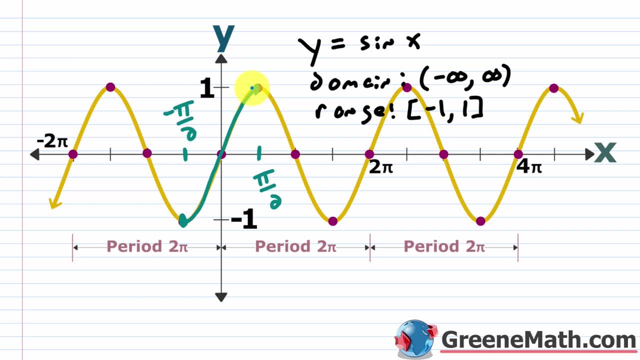 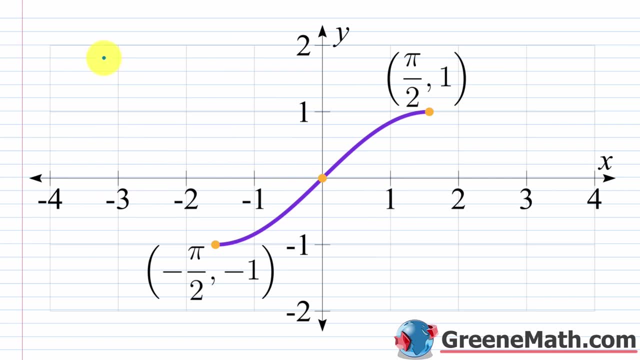 pass the horizontal line test. So it'll be a one to one function. it'll have the same range from negative one to positive one. So let me come to this graph here. it's a little bit easier to see things. So this is called the restricted sine function. So basically it's your sine function. 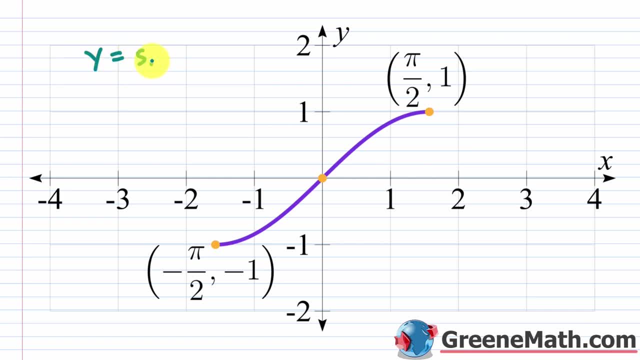 with a restricted domain. So we have: y is equal to your sine of x, And then we would say that x is greater than or equal to negative pi over two, and then less than or equal to pi over two. So obviously the domain is from negative pi over two to pi over two with. 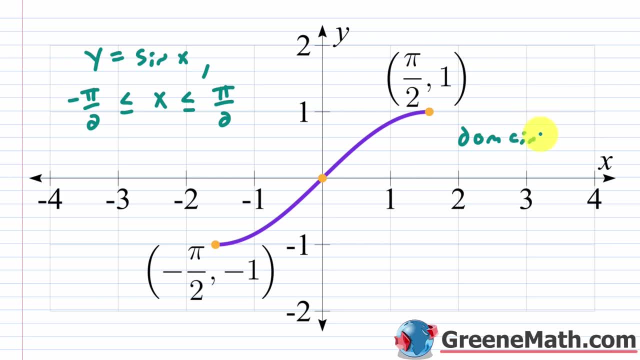 those guys included. Let me just write this out. So the domain is going to be from negative pi over two to pi over two, with both of those guys being included, And this is the key here- the range is the same. So if you go back to the y equals sine of x, again the range is from negative one to 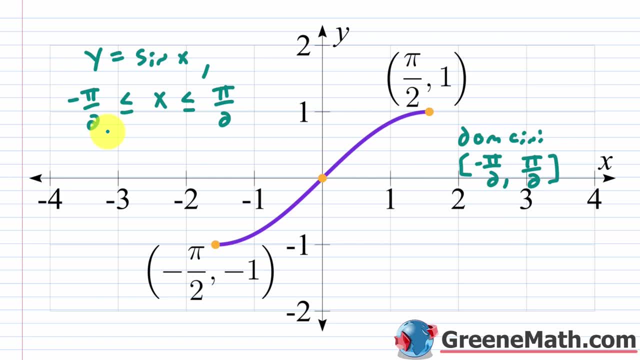 positive one. Well, here, even though we've restricted the domain, the range remains from negative one to positive one. So let me write that the range is going to still be from negative one to positive one. Okay, so now let's cover the inverse sine function. So we're going to start with the 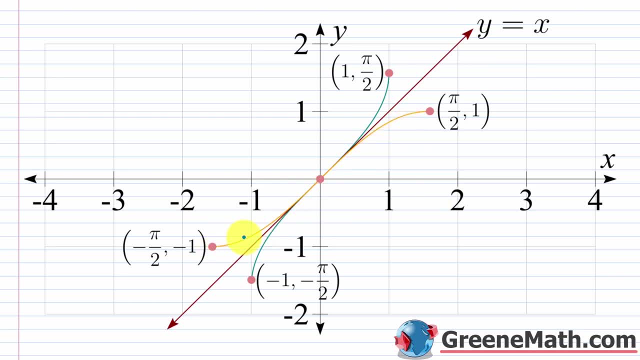 restricted sine function. So that's going to be this graph in orange. let me just trace over with the computer drew here. So this is my graph in orange. a lot of stuff is overlapping here. So this graph again is: y is equal to my sine of x, where x is greater than or equal to negative pi over. 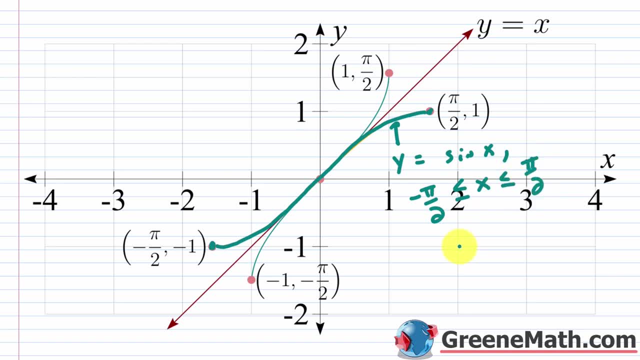 two and less than or equal to pi over two. So that's the restricted sine function. If you reflect it across the line, y equals x. you're going to generate this graph here in green, So let me go over that. So from here to here. so a lot of overlap here. you can do this on Desmos if you. 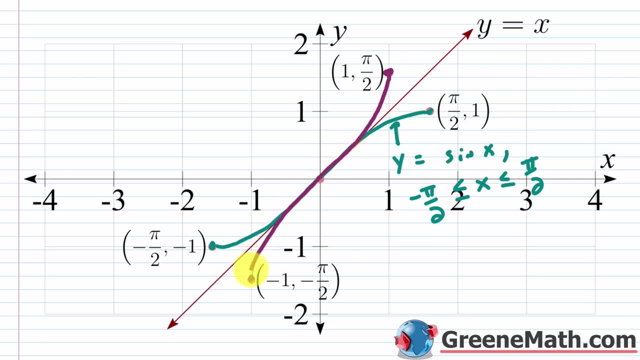 want a cleaner picture, But in terms of the video I think it's going to come through at least good enough to where you can see what's going on. So this right here is going to be the graph of the inverse sine function. Typically you'd write that, as y is equal to the inverse, 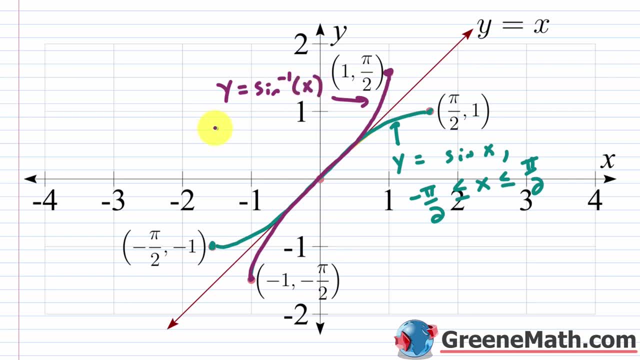 sine of x. like that, You could also write this as: y is equal to the arc sine of x, Although if you're in a trigonometry course, this is typically more common, but some books use this. it just depends, So you need to know both of those in case you run into one and not the other. Okay, so 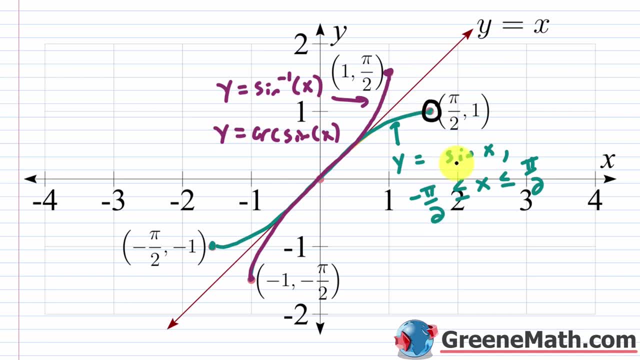 let's go ahead and take a look at the inverse sine function. So notice that this x value of pi over two becomes the y value of pi over two here in the inverse, and the y value of one becomes the x value of one in the inverse. We can also take this point right here and again reflect it across the 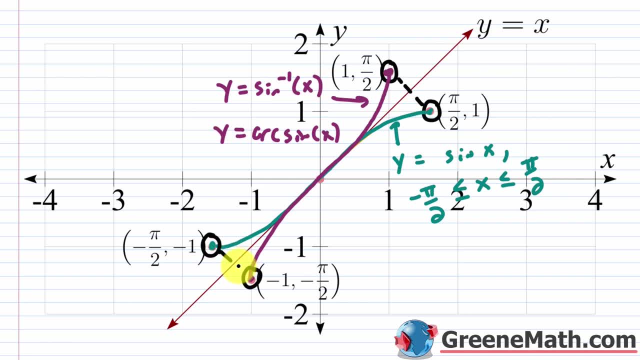 line y equals x, to get this point right here. So you see, this x value of negative pi over two becomes the y value of negative pi over two, and then the y value of negative one becomes the x value of negative one. Okay, so let's look at a. 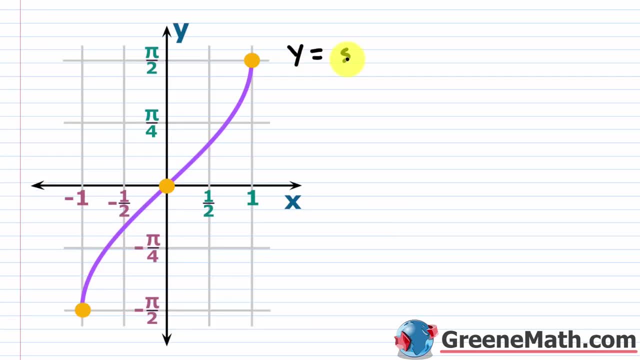 cleaner graph here. So this is the graph of y is equal to your inverse sine of x, And you can see that the domain of this guy came from the range of your restricted sine function. Let me actually put a little border here And let me write: y is equal to the sine of x, And let me put that x is greater. 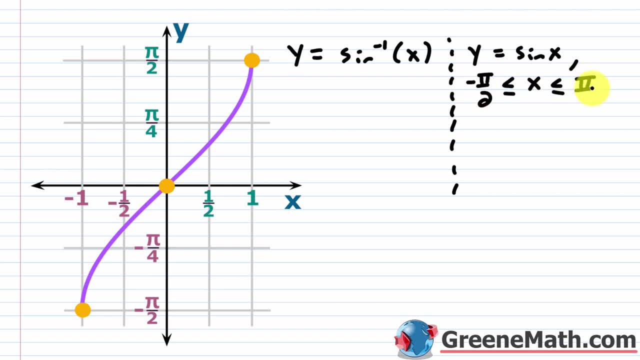 than or equal to negative pi over two and less than or equal to pi over two. And let's consider that the domain of this guy, so the domain of this guy, is the same as the range from this guy. So the domain here is from negative one to positive one. So this is going to be from negative one to 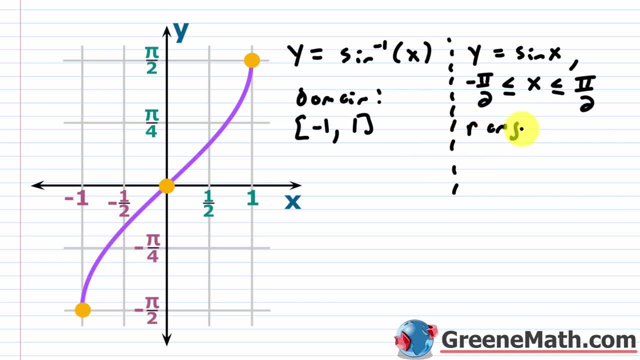 positive one. Well, here if you look at the range, if you look at the range, it's from negative one to positive one. Then if we think about the range for this guy, so the range, this is coming from the domain of the restricted sine function, So it's going to be from negative one to positive one. 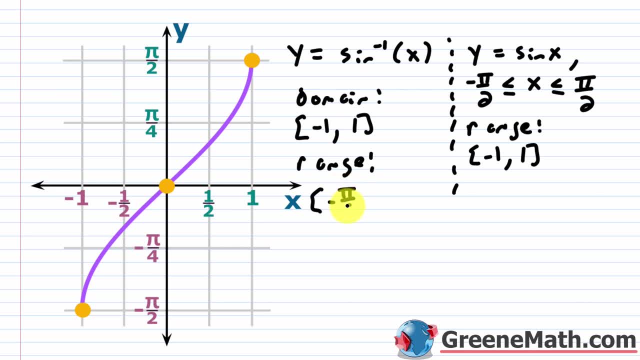 So from negative pi over two to pi over two. So from negative pi over two to pi over two. And then the domain here of course we know this at this point, let's just write it one more time. So again, this is from negative pi over two to pi over two. So just like we talked about the domain, from the 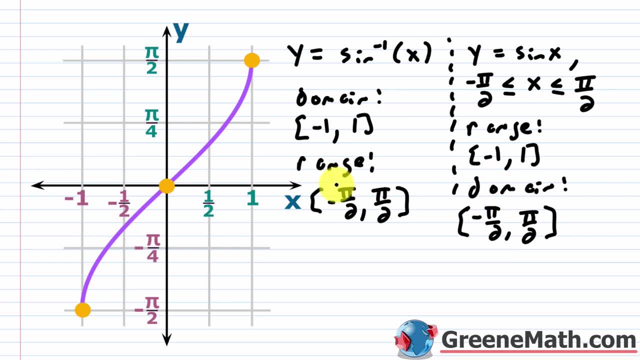 restricted sine function becomes the range in the inverse, And then the range in the restricted sine function becomes the domain and the inverse. So the x's become the y's and the y's become the x's. All right, now let's look at a few sample problems. So we're going to start with. y equals the inverse sine of. 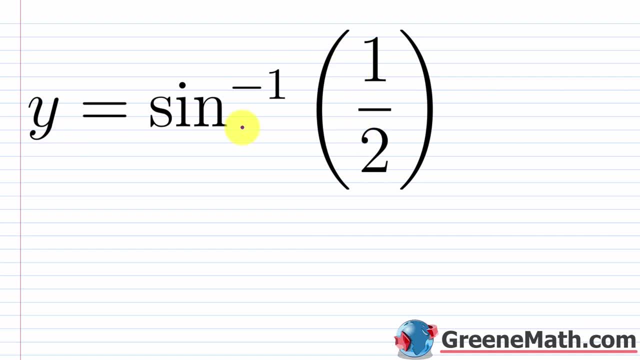 one half. So we just want to figure out what is the value for y here. So if you were to key this into your calculator, so if you were to type in the inverse sine of one half, you would get pi over six if you're working with radians, or you would get 30 degrees if you had it set to degree. 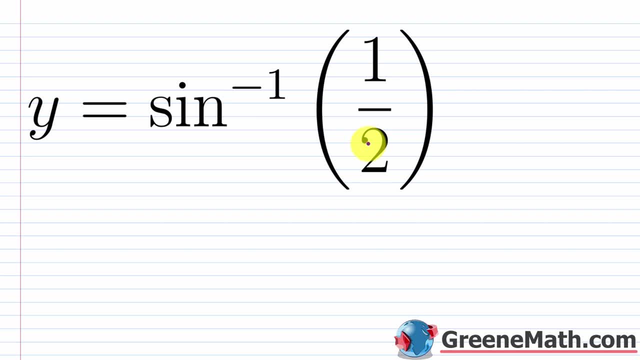 mode. So why does it give you that answer? So why does it give you pi over six and not the five pi over six that you would see on the unit circle? So we can see that for pi over six I have a sine. 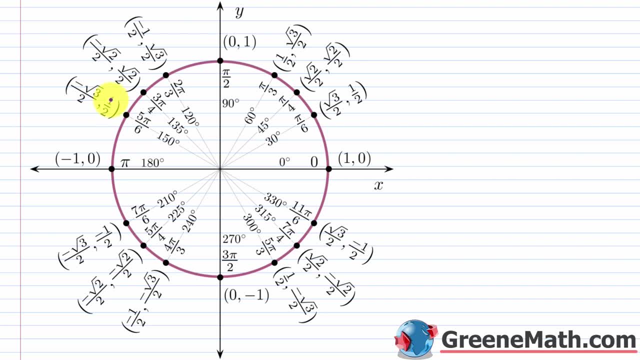 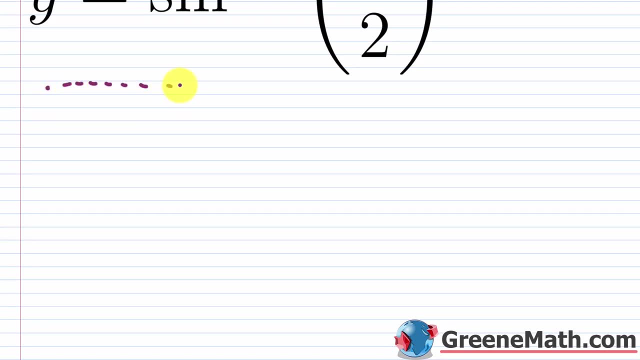 value of one half. Also, for five pi over six, I have a sine value of one half as well. Well, what's going on? Well, to see this, let's think about deriving the inverse algebraically. we saw a graphical 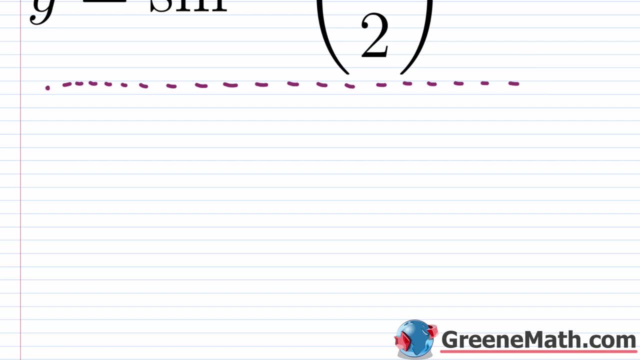 representation of it. But now let's do it algebraically And we'll get a little bit more insight into what's going on. So let's say you start with again: y equals the sine of x, And of course we need to make this one to one so we can have an inverse, So x is greater than or equal to. 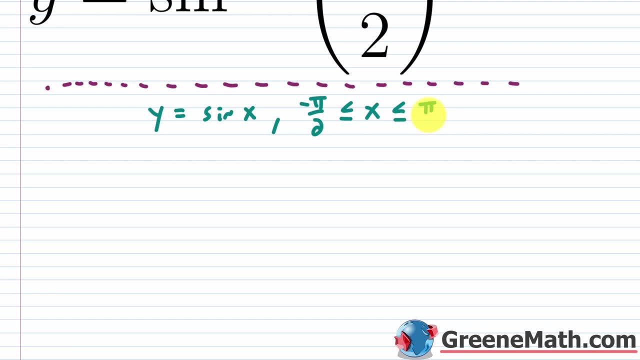 negative pi over two and less than or equal to pi over two. So to find the inverse, if you had f of x, you change it to y- well, that's already done for us here- And then basically you'd swap x and y. So this y becomes x, and it's equal to the sine of this. x becomes y. Okay, 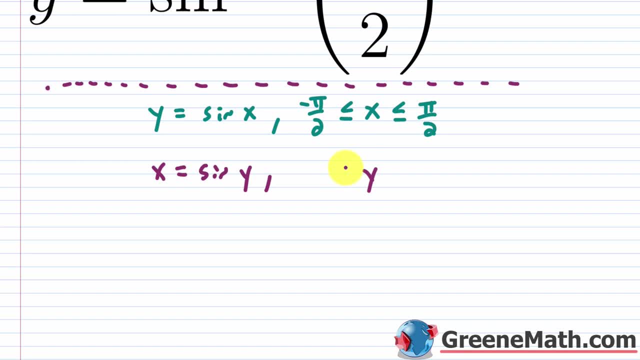 well, now this domain is going to become the range. So this is: y is greater than or equal to negative pi over two and less than or equal to pi over two. Now, this is a form that you're going to see in your textbook. what they'll say is: from here, in order to solve it for y, we're just going. 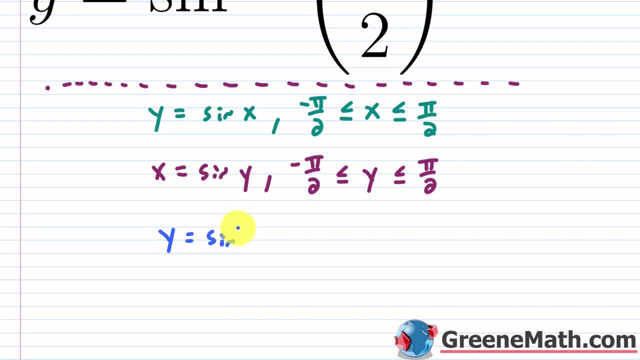 to say that it's y is equal to the sine of x. So we're going to say that it's y is greater than or equal to the inverse sine of x. So this right here is just solved. for y it means the same thing. 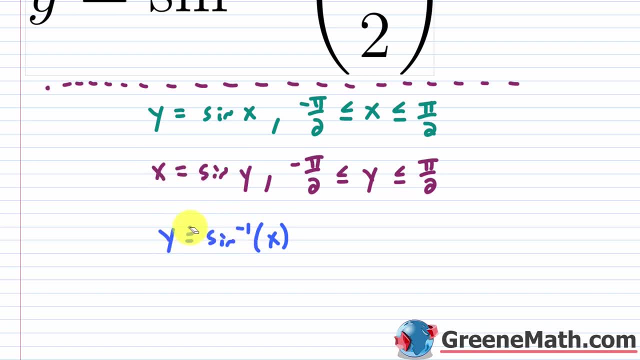 as this. Now I'm going to concentrate on it in this form for right now it's a little bit easier to think about it. So basically, let's say that we start with this right here. So the domain restricted sine function. we know that a point on that graph is going to be pi over six comma. 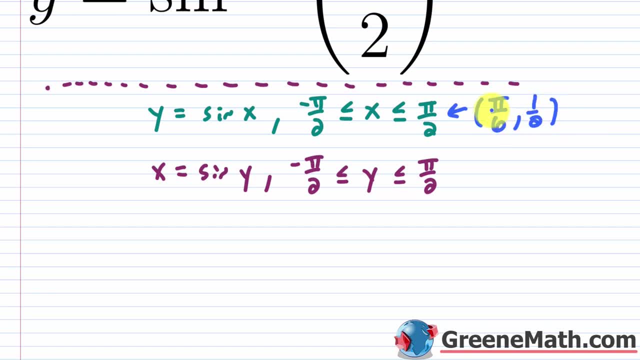 one half. So where did I get that from? Well, first off, pi over six is within the domain. it's greater than or equal to negative pi over two and less than or equal to pi over two. So if I plug that in for x, I get a true statement. So it's within the domain and the sine of pi over 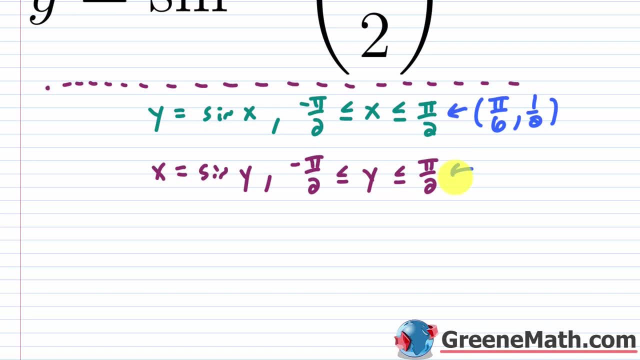 six is one half, So this would be a point on the graph. Well, when I get to the inverse, these are switched. So now this is one half comma, pi over six. In other words, when I look at this guy I am asking the question. let's say I plugged in a one half here for x. I'm saying 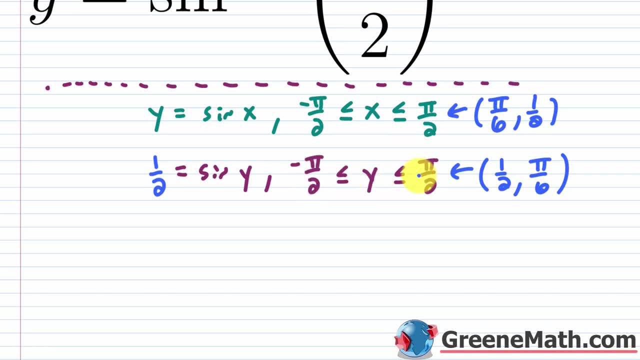 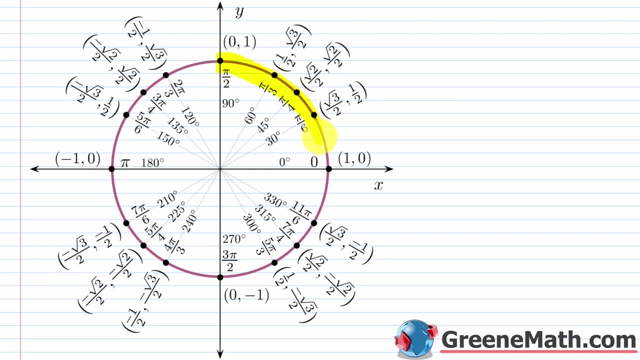 what angle in the interval from negative pi over two to pi over two is going to have a sine value of one half If we go to the unit circle? I'm going to look at this right here. So this is what I'm looking for right here. So this is pi over. 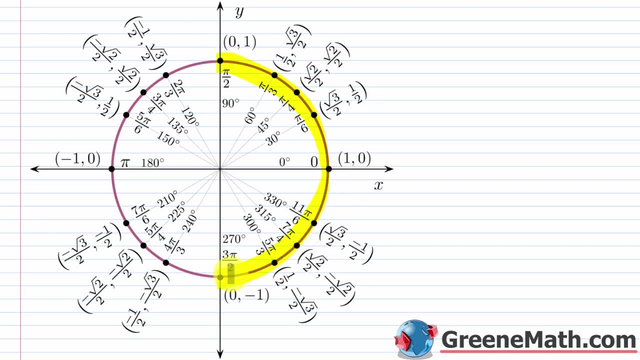 two And then this down here. if you're rotating clockwise, this is going to be negative pi over two. So this is what you're looking for here. If your argument is positive, like we have here, we're going to be looking at things in quadrant one. If your argument is negative, you're going 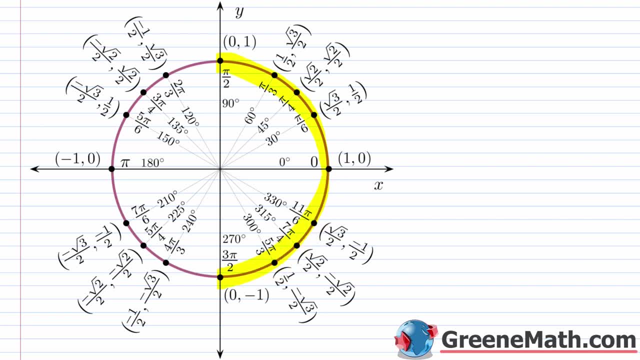 to be looking at things in quadrant four. Now there's an exception to what I just said: If you have the inverse sine. so if you have the inverse sine of one, that's going to give you pi over two And of course that's a quadrantal angle. If you had something like the inverse sine, 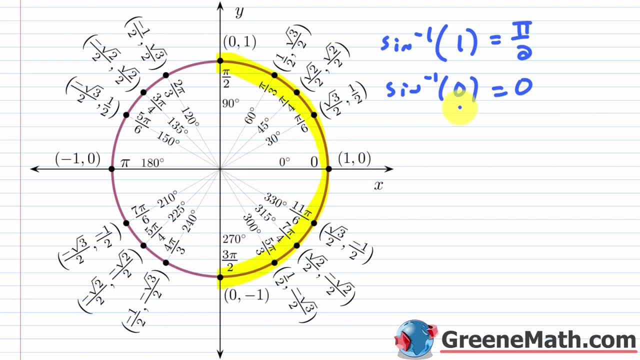 of zero, that's going to give you zero. So zero is not a positive number. But if you plug that in you're going to get something that's a quadrantal angle. And then also the inverse sine of, let's say, negative one. that's going to be negative pi over two And that's coterminal with three pi over. 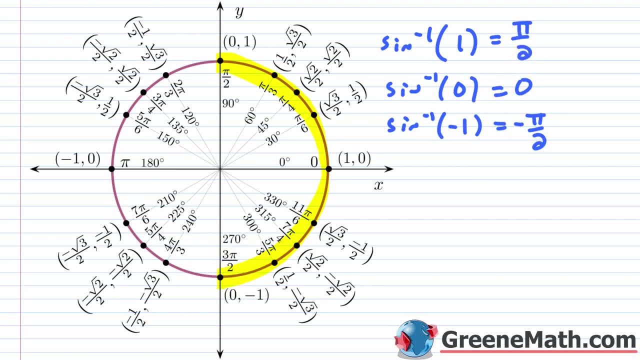 two. So again these are quadrantal angles. But if I say something like the inverse sine function is going to give you something in quadrant one if the argument is positive and quadrant four if the argument is negative. you need to just know these exceptions. Let me get rid of. 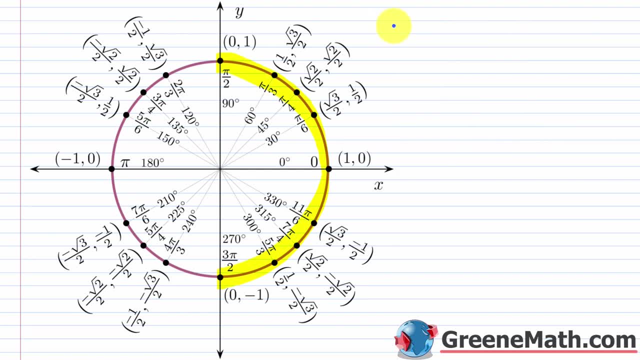 let's go back to what we were talking about. So here we have the inverse sine. So y equals the inverse sine of one half. or we wrote this as: x is equal to the sine of y, where, specifically, y is greater than or equal to negative pi over two and less than or equal to pi over two. So again, 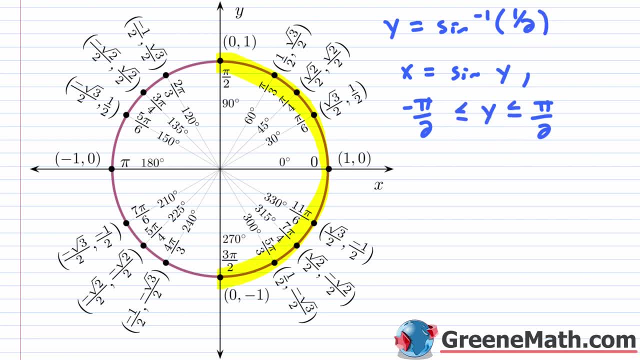 where in this interval am I going to have a sine value of one half? Well, again, this argument is positive. So I'm only going to look in the first quadrant And I see that I have a sine value here of one half. And that is going to be right here at pi over six. So that's why I'm getting this pi. 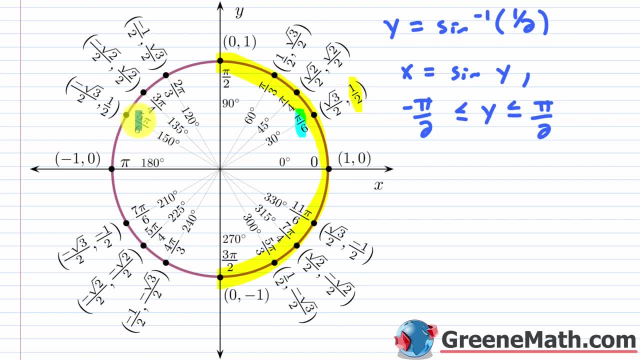 over six And I'm not getting this five pi over six here as an answer. If you notice, you have a sine value of one half for five pi over six And a lot of students will always complain: well, why am I not getting the five pi over six? you're not getting it because it's not within the range. 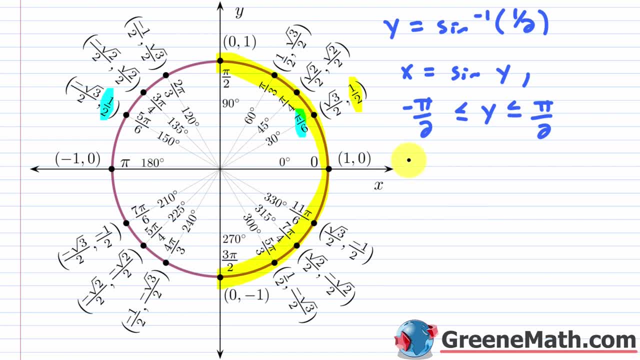 of the inverse sine function. So to answer this, if you have y equals the inverse sine of one half, let's just write: the inverse sine of one half is going to be equal to pi over six. All right, let's look at: y equals the inverse sine of a negative square root of two. 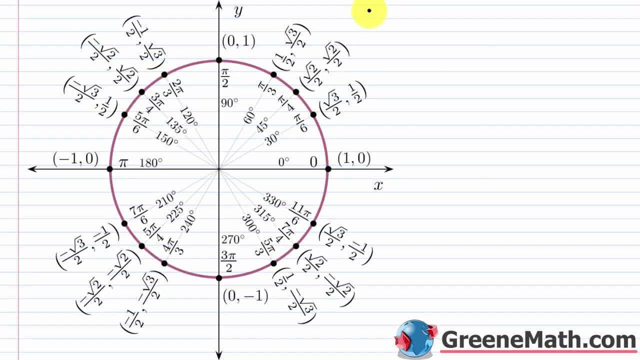 over two. So this one's a little bit more tricky. Let's come down to the unit circle. Let me write: y is equal to the inverse sine of negative square root of two over two. Again, you can stick with it in this form if you want. You're just looking in quadrant four for an angle whose sine value 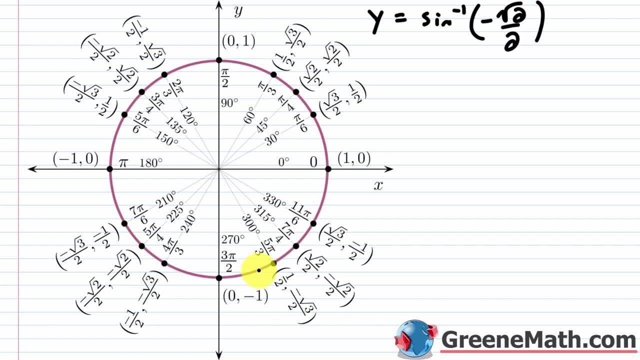 is going to be negative square root of two over two. That's what you're looking for. You can again write: y is equal to the inverse sine. of y is equal to x where y is greater than or equal to negative pi over two and less than or equal to pi over two. And of course you could just plug in a: 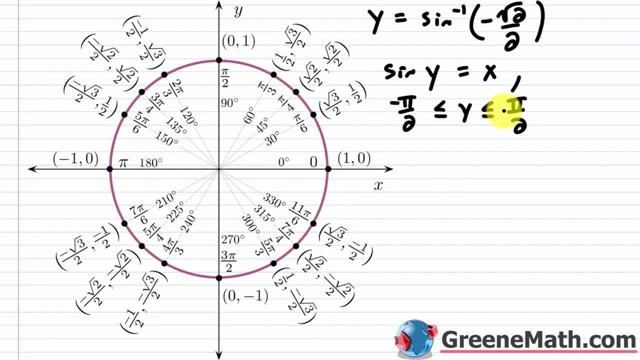 negative square root of two over two. So again, y is the angle in this interval where we have a sine value of negative square root of two over two. Now, because this is negative, I want to work in quadrant four. Let me just highlight the whole thing first. Let me highlight the whole thing. 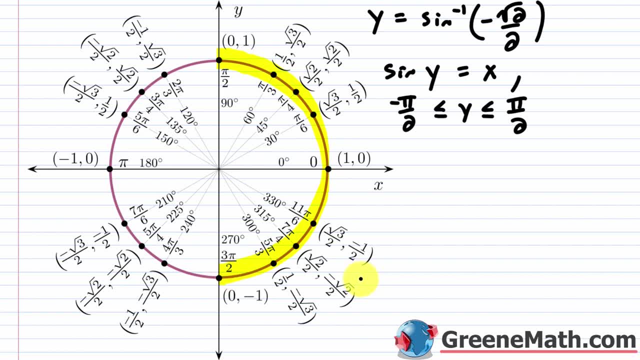 first. so we get comfortable with this. And basically, if I go into quadrant four and I'm sine value of negative square root of 2 over 2, it's going to be right there. So this is going to be at 7 pi over 4.. Now, is 7 pi over 4 the answer? No, You cannot say that the inverse sine of the 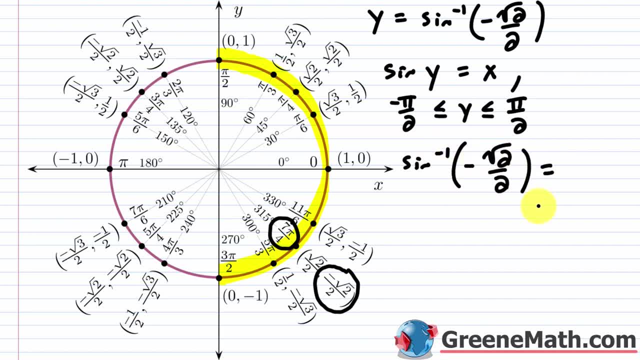 negative of the square root of 2 over 2 is equal to 7 pi over 4.. That is incorrect because it's not in this interval. What you have to do is actually rotate clockwise here. Let me pick a good color here that's going to show up. So this right here you need a clockwise rotation. So the reference. 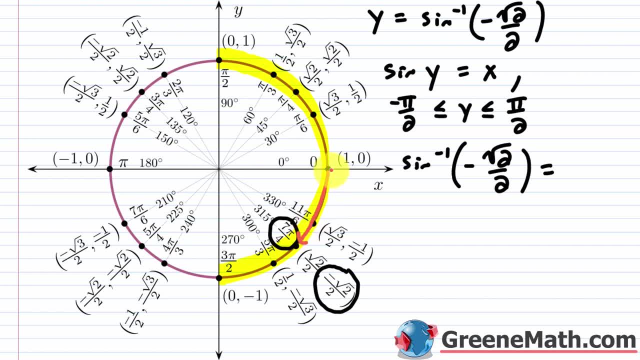 angle there is pi over 4.. So this rotation clockwise, this angle is going to be negative pi over 4.. So this would be negative pi over 4 as the answer. Now, another way you can do this. it's a longer way, but essentially what you could do is you could figure out. okay, I'm going to be 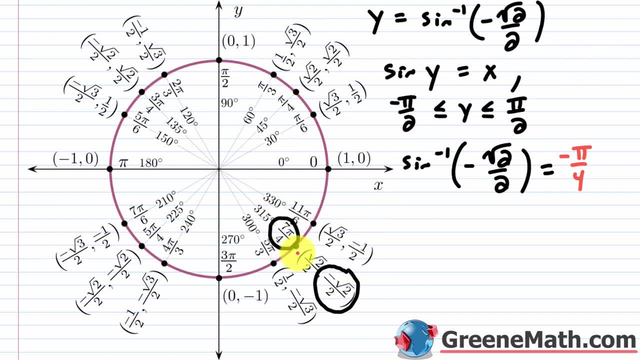 in quadrant 4.. So I want this 7 pi over 4 answer, but I need to put it into this interval. since I started here and rotated all the way around By 7 pi over 4, what I have to do is now rotate clockwise by 2 pi. So that's going to be me. 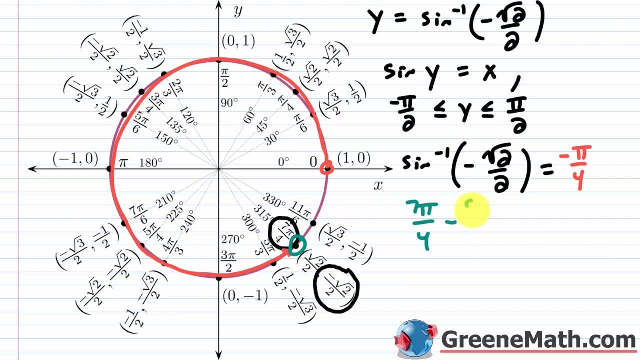 taking 7 pi over 4 and subtracting away 8 pi over 4 to get my negative pi over 4.. So in other words, you're going to go this way clockwise by 2 pi. So that's just subtracting 2 pi away, So coming. 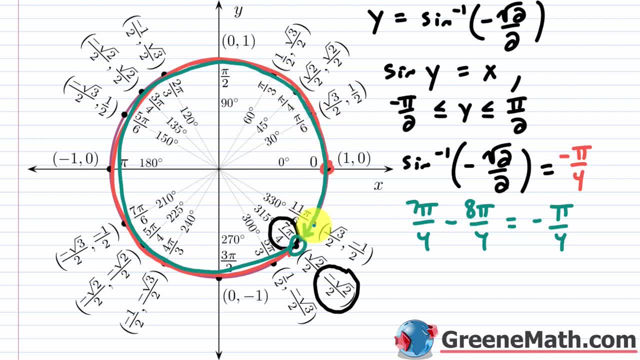 back here and finding a coterminal angle, So ending up right there. So now I get the angle that I want, which is going to be negative pi over 4.. I think this is a little bit more complicated, but sometimes people need to do that to figure. 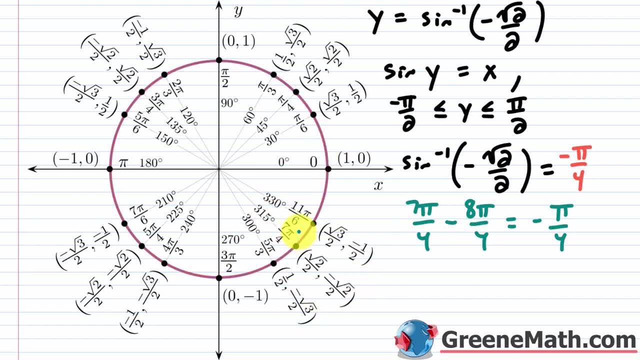 out what's going on. What I always do is figure out what the angle is, So in this case, okay, it's 7 pi over 4.. The reference angle is pi over 4 and I know it's negative, So it's just negative. 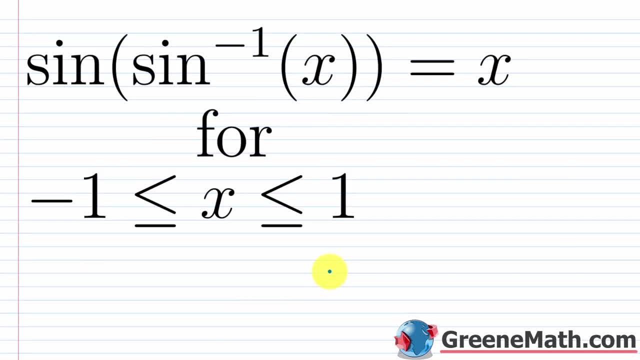 pi over 4.. I think that's pretty easy to understand. All right, now let's talk about the cancellation properties for sine. So these are some simple rules you can use to quickly evaluate things. So the first one's very straightforward. So you have something like: 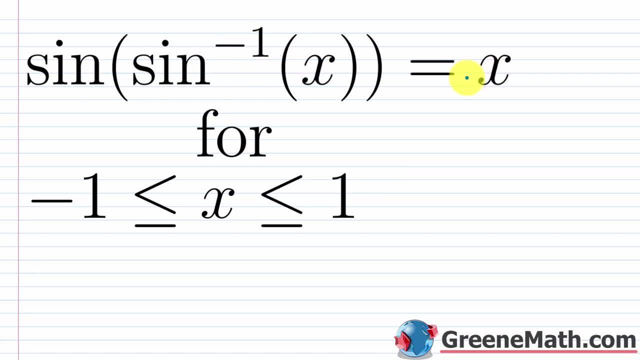 the sine of the inverse sine of x, That's going to be equal to x, for x is greater than or equal to negative 1. And less than or equal to positive 1.. So why do we need this restriction here? So, first off, if you consider the outer part here, so the sine of, so this right here is the 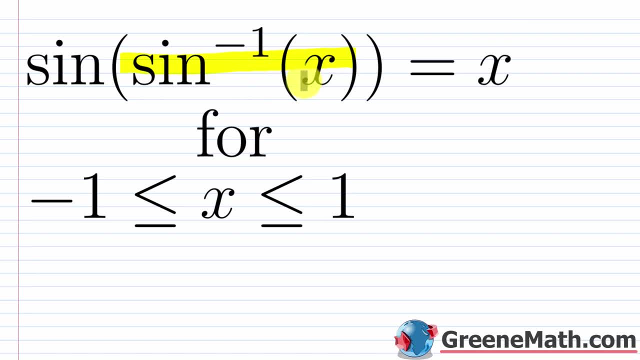 argument for the sine function. Does it matter what I plug in for the sine function in terms of the domain? No, because it's all real numbers, So I can plug in whatever I want: a negative, zero, positive, whatever I want. The problem actually comes from the inverse sine function. 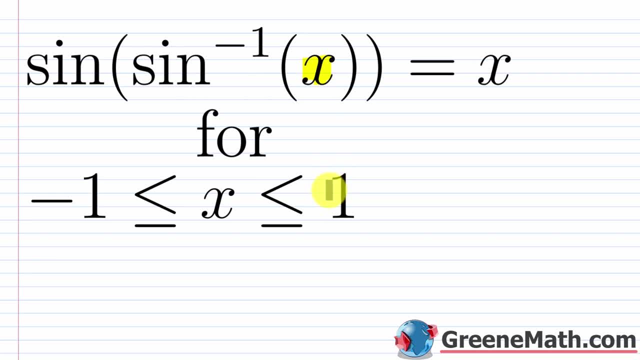 So here, if I look at this x here, what can I plug in for that? Well, remember, the domain of the inverse sine function is going to be from negative 1 to positive 1.. So that's where you have to be careful. If you did something like the sine of the inverse sine of 2, well, you're not going to be. 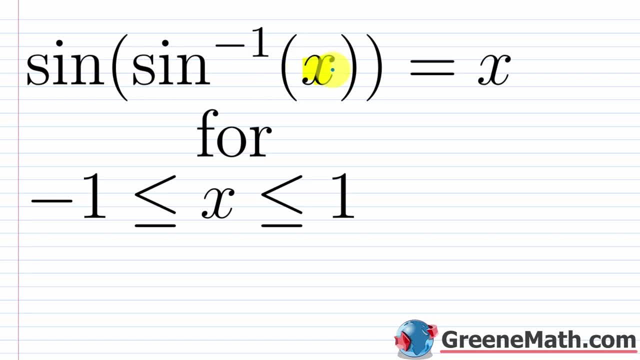 able to get an answer there, because the inverse sine of 2, you can't type that into your calculator and get an answer. It's just going to give you an error. So what you would want to do is make sure that it's within this interval here And then if you had a problem like the sine of, let's say, 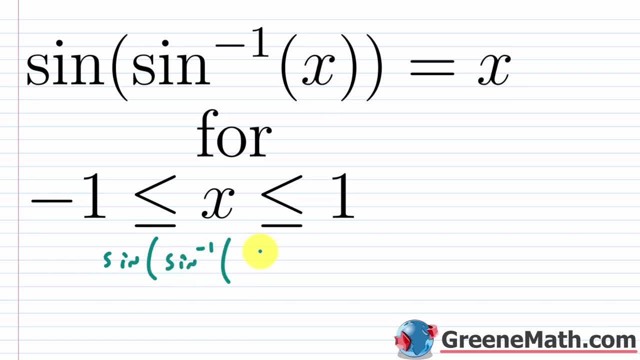 the inverse sine. and then for this let's say we go with what we just did. So let's say we plug in 1 half. Well, this let's say we plug in 1 half. So what we're going to do is we're going to plug in 1 half. 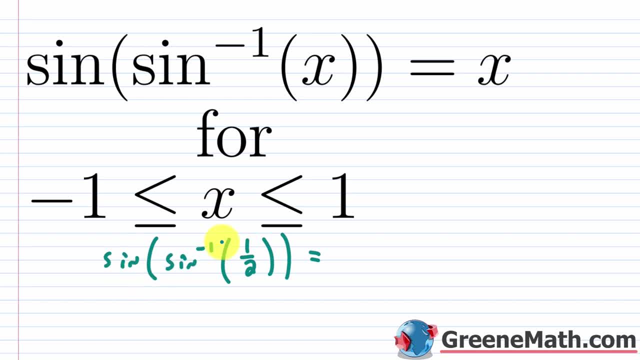 is going to just give me one half. In other words, these guys are just gonna cancel away and I'll be left with this one half If you wanna do this the long way. the inverse sign of one half- we just saw that- was pi over six. 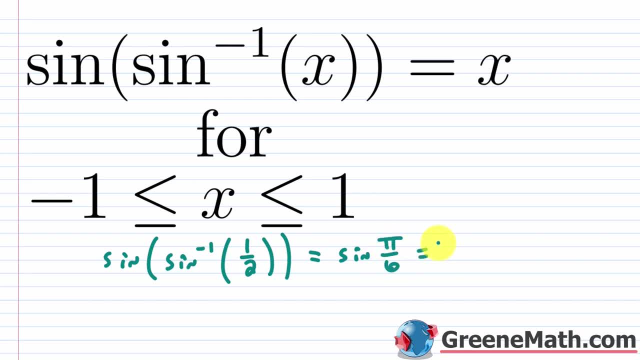 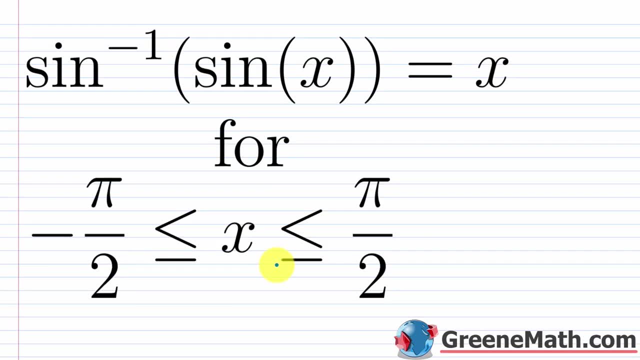 So this would be the sign of pi over six, which we know is one half. So I can just skip this step right here and just go straight to saying that the answer is one half. All right, so the next one is a little bit more challenging to understand. 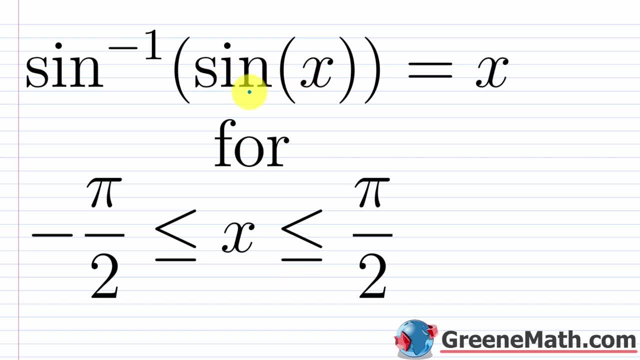 So what you wanna concentrate on is the first part. so the sign of X. So think about that for a moment. We know that, again, the domain for the sign function- this is not a restricted sign function or anything like that. I can plug in whatever I want for X. 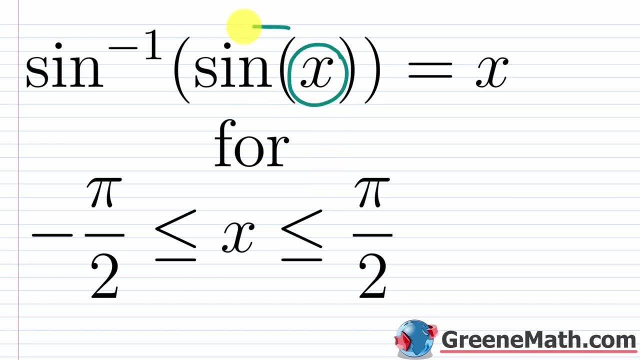 It does not matter any real number, So plug in whatever you want. The result of the sign of X is going to be from negative one to positive one. Now, with the inverse sign function, remember the domain or what you can plug in. 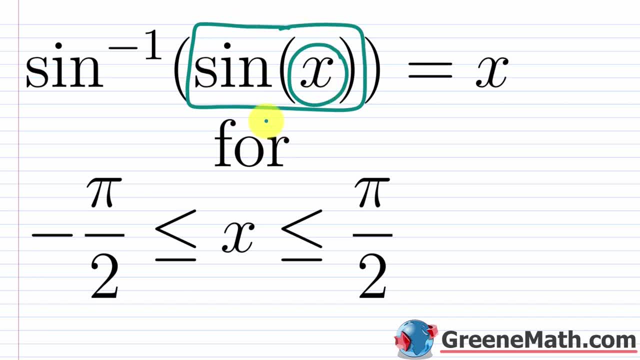 is gonna be from negative one to positive one, So I'm good to go in terms of plugging things in for the inverse sign function. I'm not gonna run into any issues. But the problem is that the range or the output for the inverse sign function 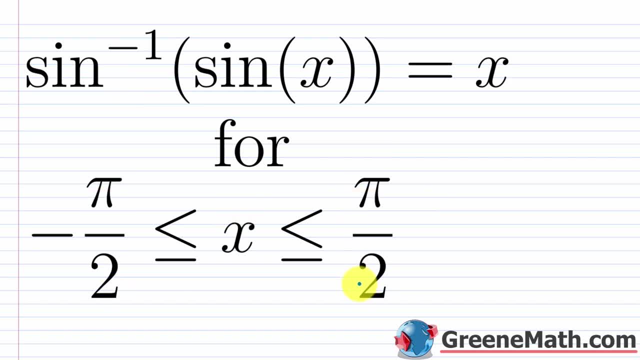 is only going to be from negative pi over two to pi over two. So if you're in that interval, you can just cancel this with this and say it's equal to X. If you're not, you need to evaluate the sign of X first. 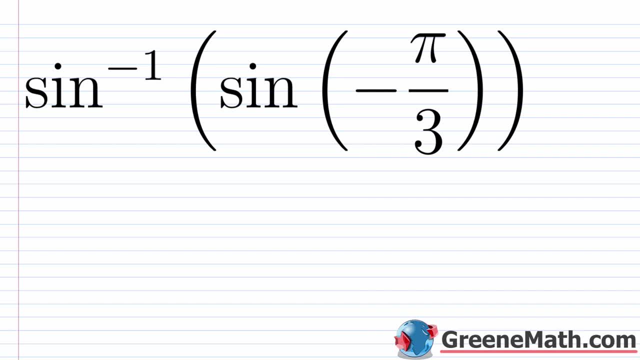 and then take the inverse sign. So let's look at two examples. So the first one is: we have the inverse sign of the sign of negative pi over three. So to answer this, the first thing you would do is say: is negative pi over three, greater than or equal to? 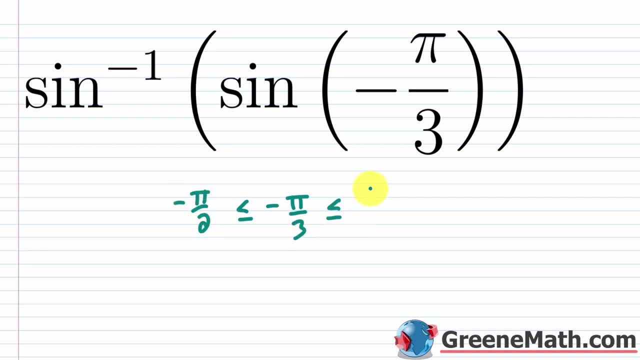 negative, pi over three, Pi over two and less than or equal to pi over two. Well, this part I know. I know that negative pi over three is certainly less than pi over two, because a negative is always less than a positive. Now, what if you compared this one? 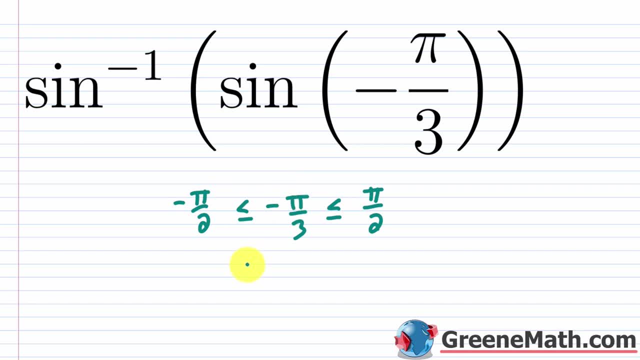 Well, the numerators are the same. Forget about the fact that they're negative for a moment. Let's say you had pi over two and pi over three, And I just put a question mark here. So if I look at this, the numerators are the same. 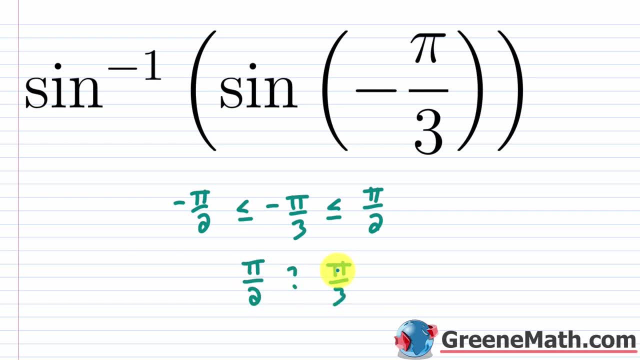 The denominators are different, So same numerator. That means that the larger denominator is going to belong to the smaller fraction. So I can say that this guy right here is greater than this guy right here. But now, if I multiply both sides by negative one, 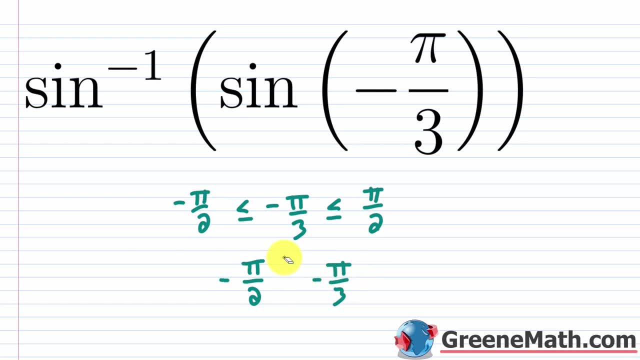 that's going to change. So this right here, this right here and this gets flipped. So now this guy, which was the larger fraction, because now that it's negative it's going to actually be the smaller fraction because it's further to the left of the number line. 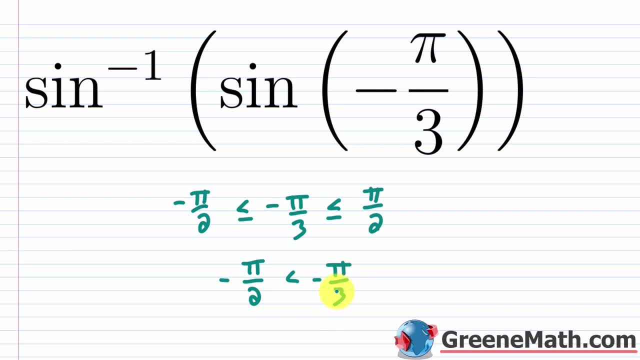 So that means that negative pi over two is less than negative pi over three. So this inequality is going to be true. So that means that I can just say that the answer here- let me slide this out of the way- is just going to be negative pi over three. 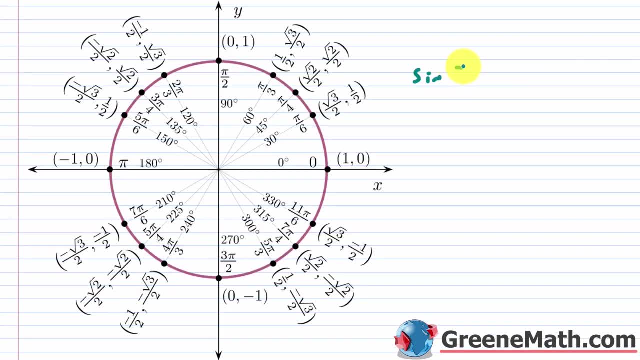 If you go to the unit circle and you want to define the sign of negative pi over three, Again, I'm just looking for an angle in quadrant four with a pi over three reference angle. So that's going to be right here at five pi over three. 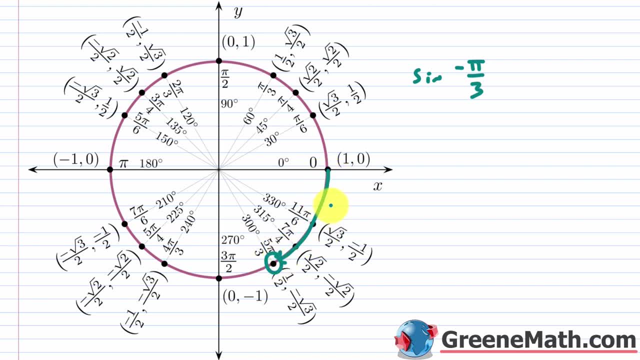 But again, I'm not thinking about it as five pi over three because I'm rotating clockwise, So that's my negative pi over three angle. So the sign of a negative pi over three is the same as the sign of five pi over three. 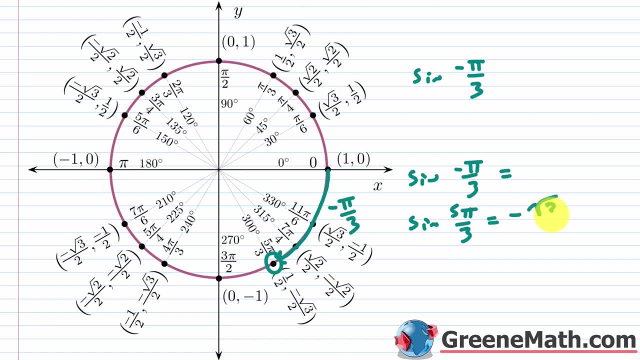 the coterminal angle. So that's going to be the negative of the square root of three over two. So if you went through and said, well, what is the inverse sign? So what is the inverse sign of the negative of the square root of three over two? 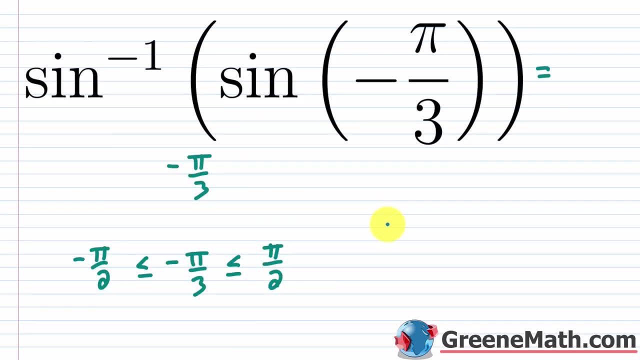 You're going to go right back to that negative pi over three. So again, if you're in this interval, you can just shortcut all that and just give this as the answer right away. So the answer here is just negative pi over three. 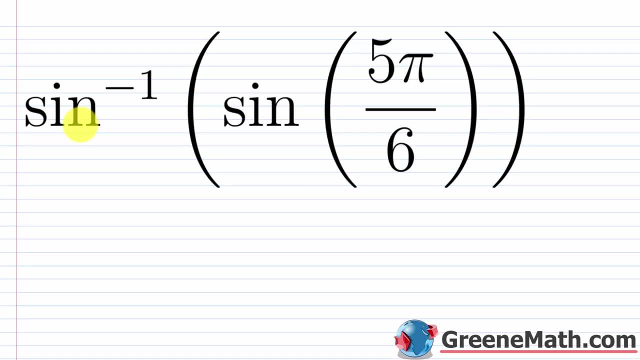 All right, let's look at another one. So this one will give us a little bit of trouble. So we have the inverse sign of the sign of five pi over six. So can we just say the answer is five pi over six? No, And the reason for that is five pi over six is not. 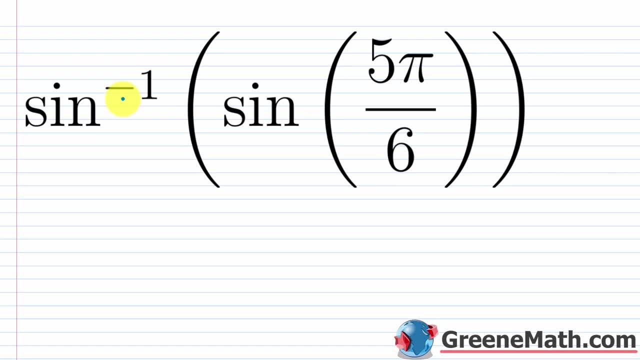 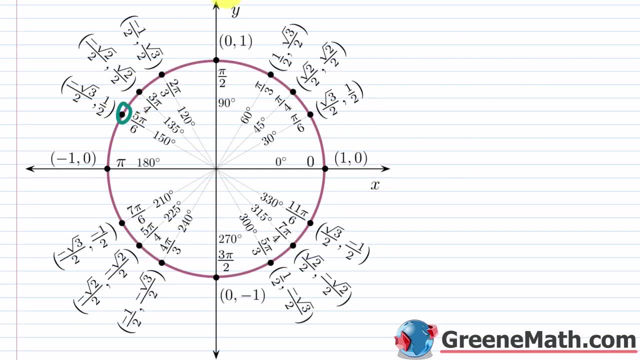 in the range of the inverse sine function. We cannot get that as an answer. So because of that again, what you'd have to do is first find the sine of five pi over six. So, coming to the unit circle, here's your five pi over six. 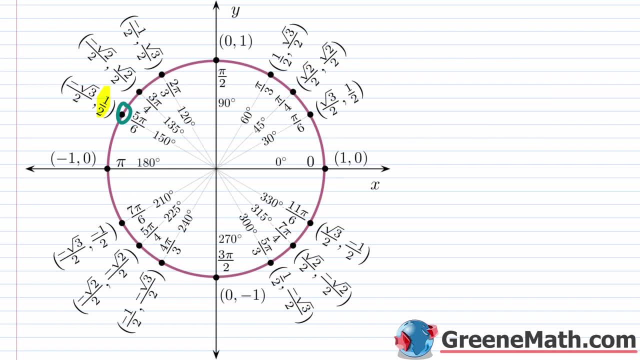 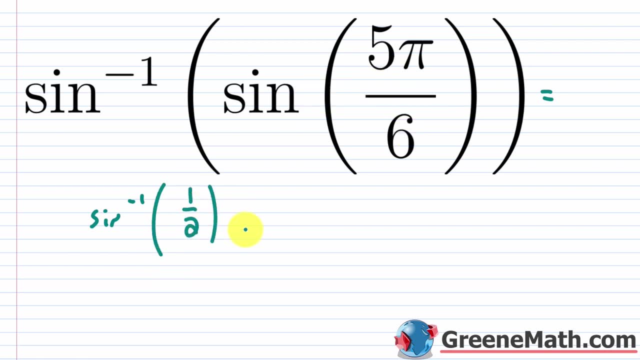 And all of you know that that's one half. So basically you would have to transform this into the inverse sine of five: pi over six is one half, And then we know that this is pi over six. But again, if we just come back down, you're working here. 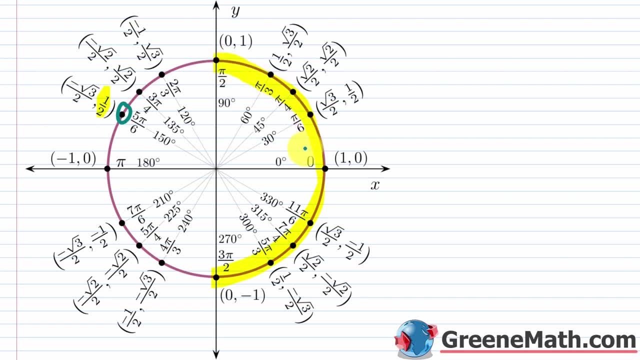 And this guy is going to be positive. So you're looking in quadrant one for an angle with a sine value of one half. So you've got that right here and that's going to be at pi over six. So that's the angle I'm looking for. 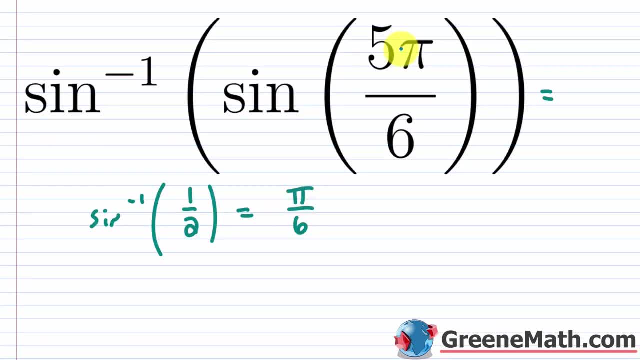 So, coming back, we just answer pi over six. So when this guy right here is not in the range. So from negative pi over two to pi over two of your inverse sine function, you've got to do additional work First. you're going to do the inside. 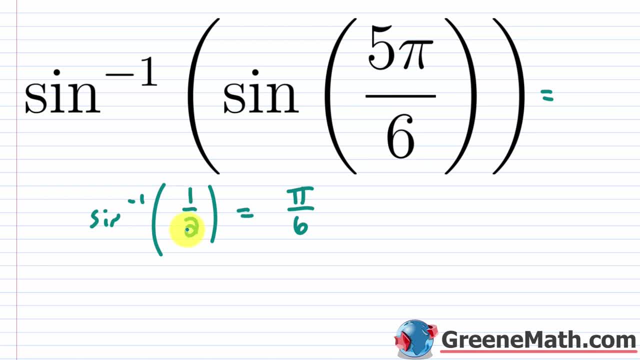 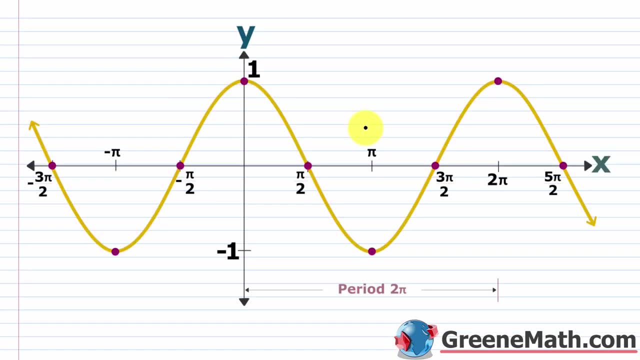 So evaluate the sine of five: pi over six, That gives me one half. Then take your inverse sine of one half, and that's going to give me pi over six. All right, Now let's move on and talk about finding the inverse cosine function. 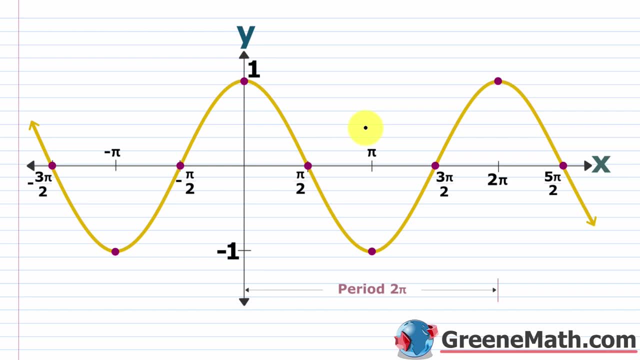 So the process is exactly the same as what we did for finding the inverse sine function. There's just a few differences in terms of what part of the graph we're going to take in order to create a one to one function. So we would start with the graph. 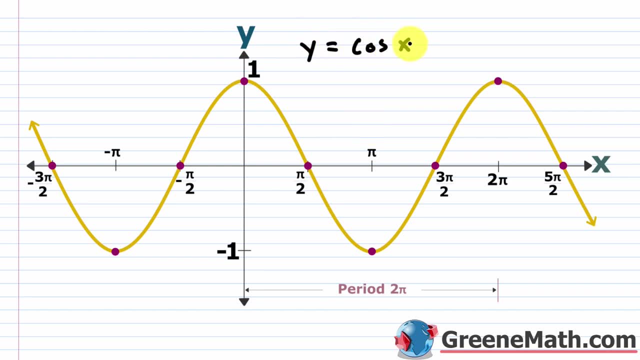 of y is equal to the cosine of x. So we've studied this graph before. We know that the domain is all real numbers and the range is from negative one to positive one. So let me write here that the domain is going to be the set of real numbers. 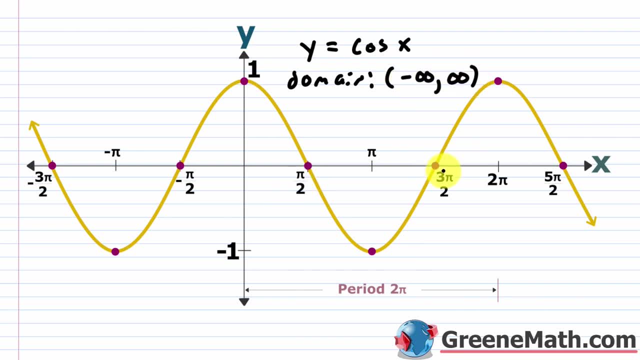 So from negative infinity to positive infinity. So I can plug in whatever I want for x there. So a negative zero, a positive, whatever I want, as long as it's a real number. And then for the range. So for the range we can see that this is from negative. 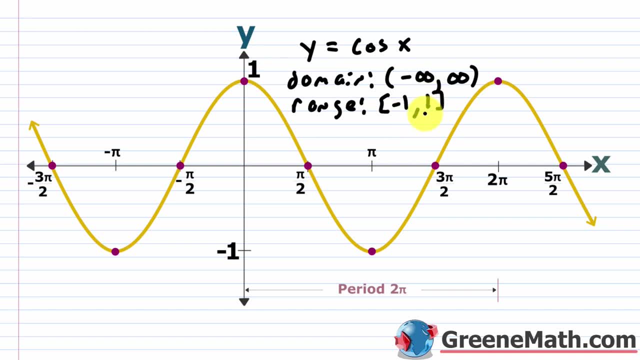 one to positive one, with both of those being included. Now again, this function is not a one to one function. You can see that from the graph. If I make myself a little horizontal line here, you're going to see that it hits here and then here, and then here and then here. 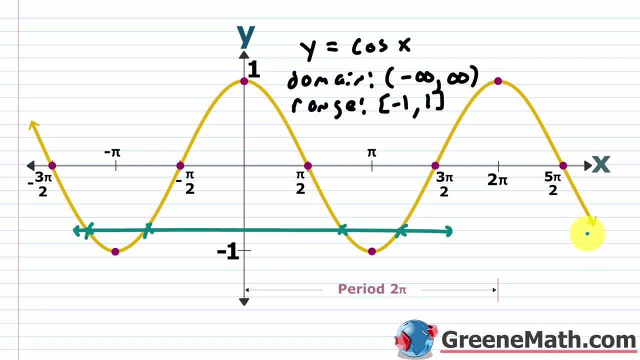 And again, this graph continues forever to the right and forever to the left, So it's going to keep hitting over and over and over again. So obviously this is not the graph of a one to one function. So again, what do we do? 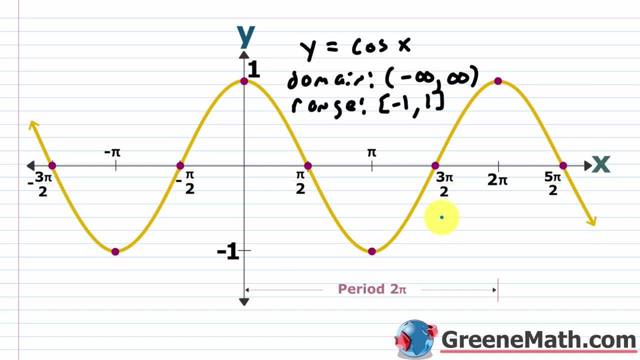 Well, we're going to restrict the domain such that we have the same range. So for this one, what we want to actually do is start at zero, so an x value of zero, and then go to an x value of pi. So this is the piece of the graph we want. 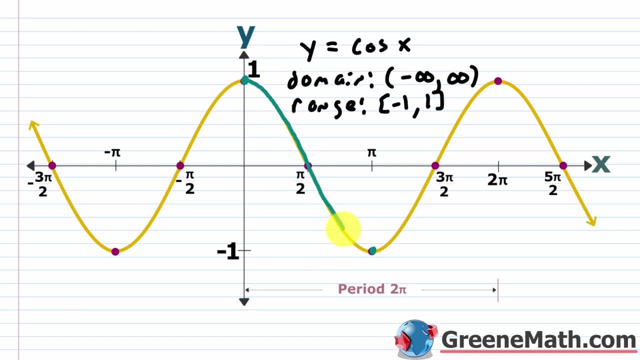 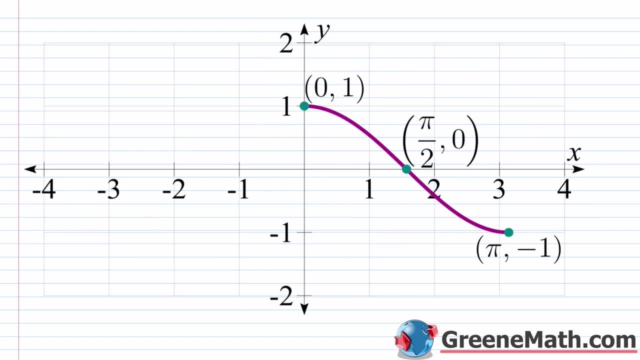 So this is going to be from zero to pi, And notice that your range is not going to change: It's still going to be from negative one to positive one. So this would create a one to one function for us. And, to see that more clearly, this is the graph of our restricted cosine function. 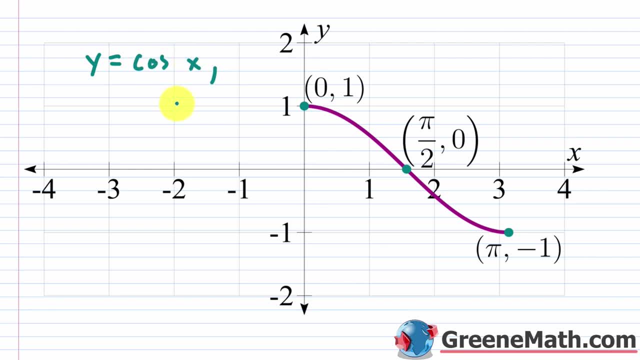 So this is: y is equal to the cosine of x, where x is greater than or equal to zero and less than or equal to pi. So you can see this would be a one to one function. now And let me just write here for clarity that the domain, obviously it's right here. 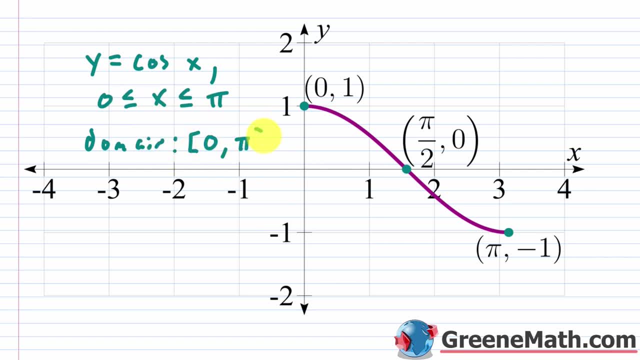 But let's just list it. So this is going to be from zero to pi, where zero and pi are both included, And then the range- This is the key here. It's going to be the same as your regular y equals the cosine of x. 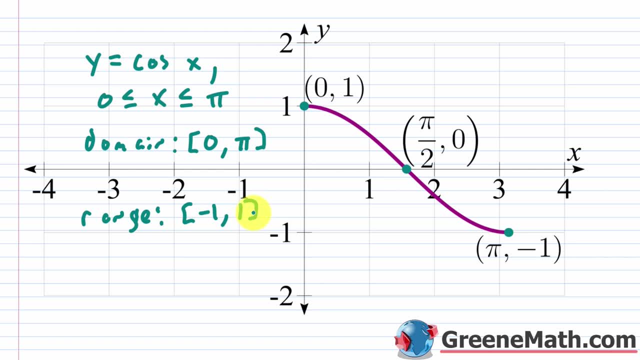 So it's still going to be from negative one to positive one, with both of those guys being included. Now what we can do if we want to find our inverse is reflect this graph across the line y equals x. So if we start with this graph again in purple, this is the graph from the previous. 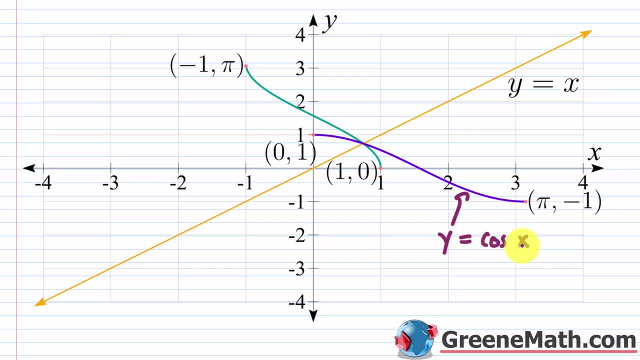 page- this is my- y is equal to the cosine of x, where x is greater than or equal to zero and less than or equal to pi. So again, the restricted cosine function. Let me just go over this for clarity. So this graph right here again you're going from zero to pi and the range 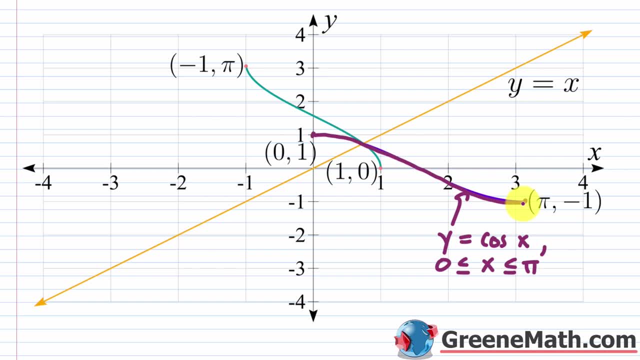 And this is the key- is still from negative one to positive one. So when you reflect this across the line, y equals x. that's this guy in orange. here you're going to get this graph. that's in teal. So this guy right here is the graph, for y equals the inverse cosine of x. 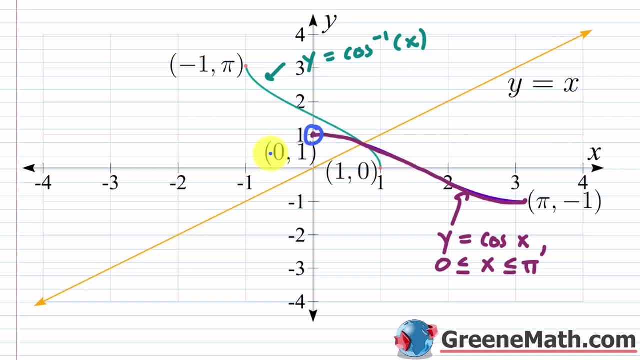 So if you started with something like: let's say this point right here, which is zero comma one, And you reflect across the line y equals x, You're going to get to this point right here, which is one comma zero, And that's going to be on your inverse. 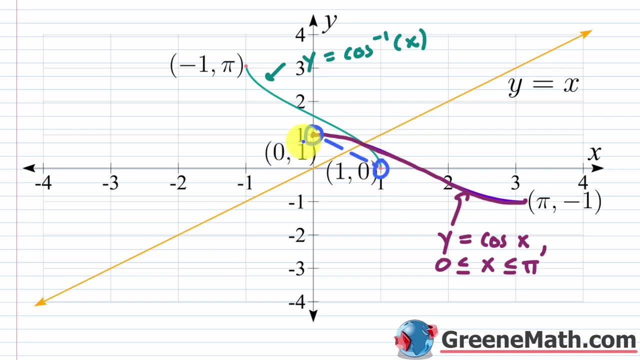 So the x value of zero becomes a y value of zero, And then a y value of one becomes an x value of one. So those x's and y's are switched. Then if we look at this other point right here, which is pi comma, negative one, 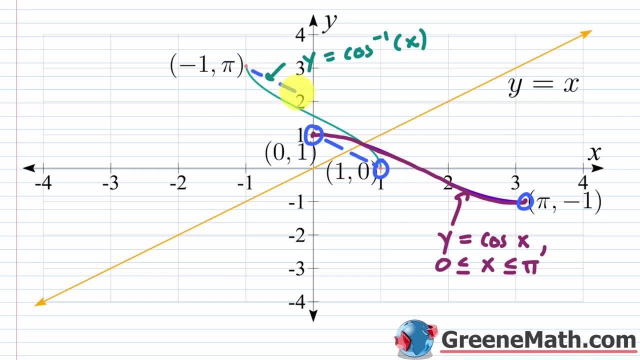 Again, if I reflected across the line, y equals x- I'm going to get this point right here- which is negative one comma pi. So here the x value of pi becomes the y value of pi in the inverse, And then the y value of negative one. 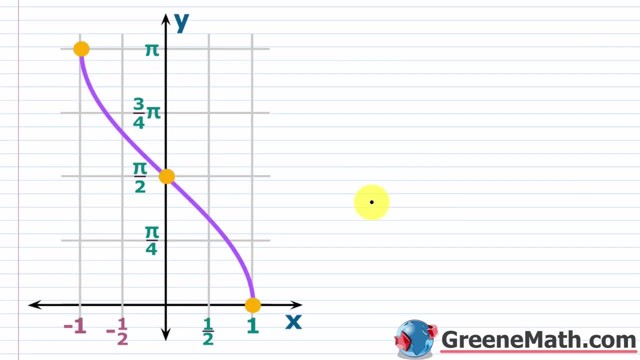 becomes the x value of negative one in the inverse. To get a better look at this, we can see this graph on its own. So this is for y is equal to your inverse cosine of x, And let me put a little border, Just like we did last time. 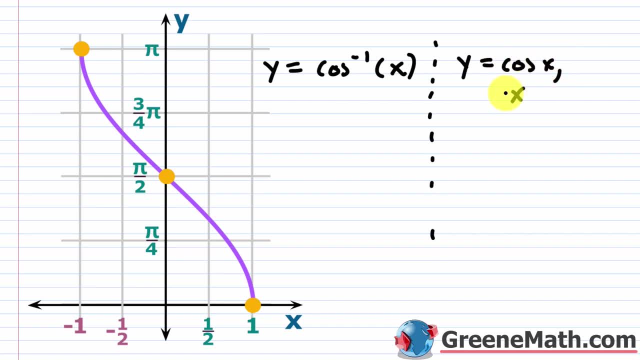 Let me put: the y is equal to the cosine of x, where x is greater than or equal to zero and less than or equal to pi. And again for this one, we know that the domain. So we know that the domain because it's listed specifically right here. 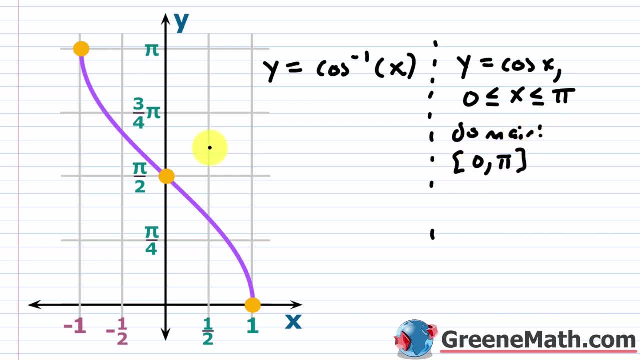 is going to be from zero to pi. Well, notice that the range here for the inverse cosine function is going to be from zero to pi. So let me write that the range for this one is going to be from zero to pi. So the domain becomes the range. 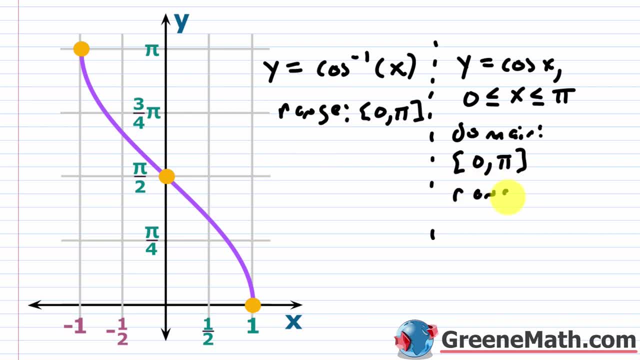 And the range is going to become the domain. So the range here, So the range in this case is going to be from negative one to positive one, And you're going to see in the inverse again, the domain now is from negative one to positive one. 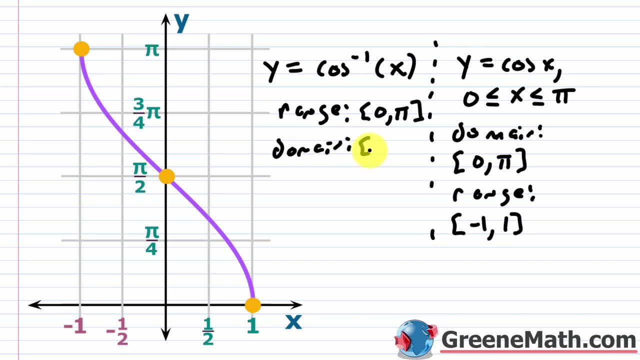 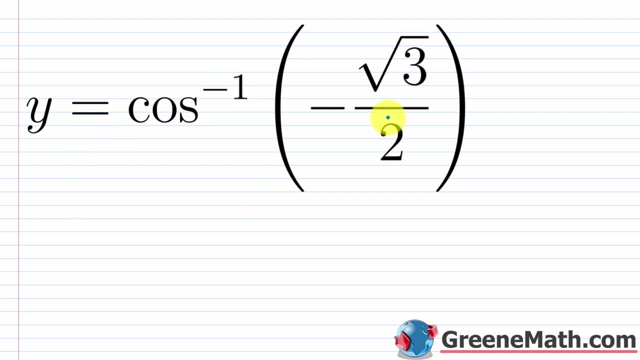 So let me put that: the domain Is from negative one to positive one. All right, let's look at a few problems now. So here we have. y equals the inverse cosine of the negative of the square root of three over two. So again, a lot of you can immediately say that the answer is going to be five pi over six. 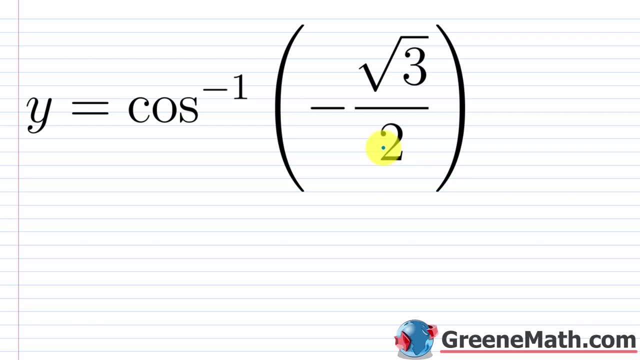 But just to go through this the long way, so we understand where this stuff is coming from, What we want to do is think about this: y equals the cosine of x, So just start with this, like we did graphically, And we're going to restrict the domain. 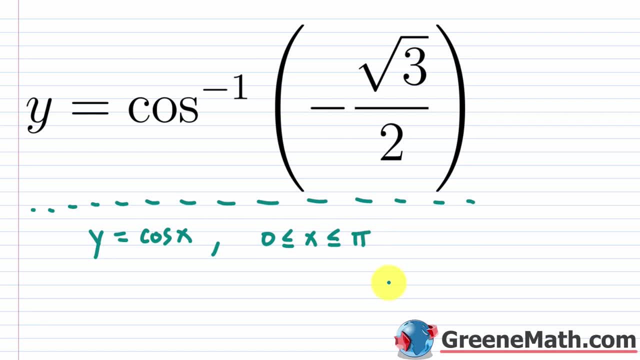 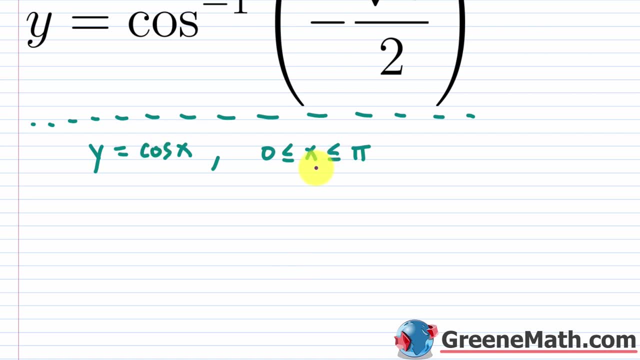 So x is greater than or equal to zero and less than or equal to pi. If you go through, this is going to get cut off, So let me just slide down here. We'll come back up. So if you go through and find the inverse of this domain restricted function, 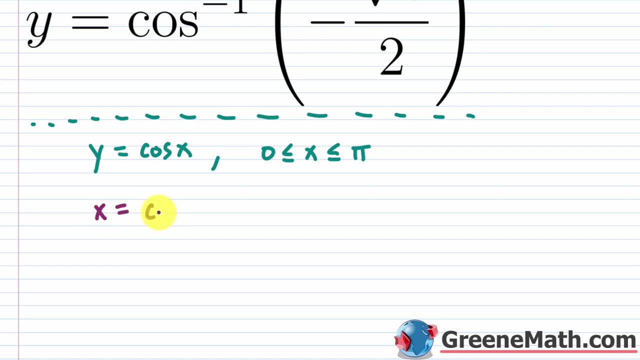 you swap the x and the y, So you end up with: x is equal to the cosine of y And of course this right here, which is the domain, becomes the range. So now you have: y is greater than or equal to zero and less than or equal to pi. 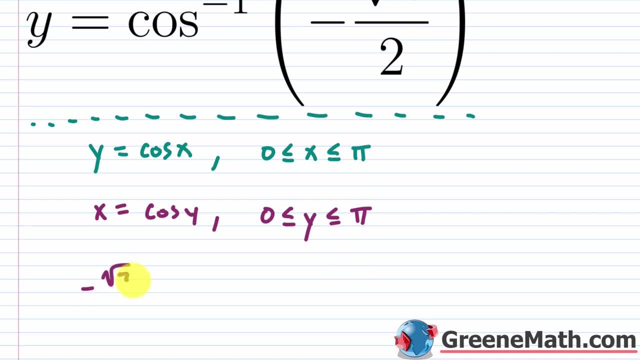 So if I have something like: let's say, the negative of the square root of three over two is equal to the cosine of y, where y is greater than or equal to zero and less than or equal to pi. Well, when it's written this way, 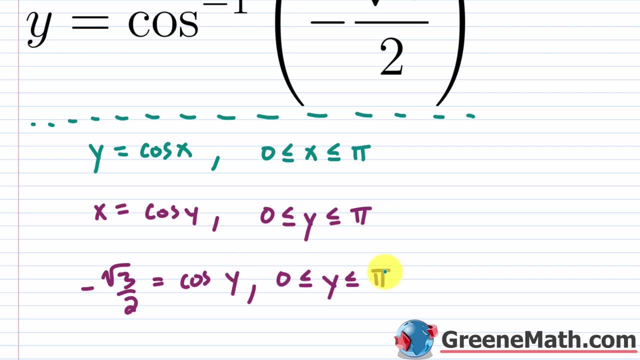 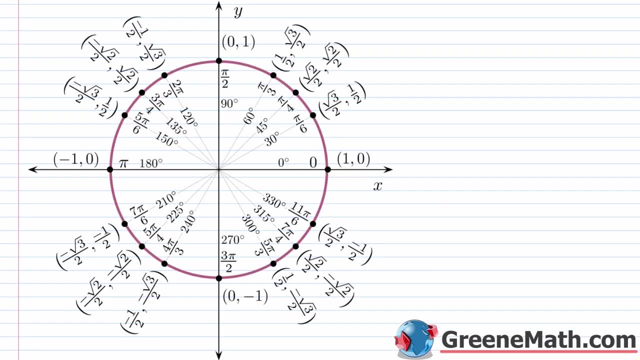 you can say that y is going to be the angle between zero and pi, where zero and pi are included, where your cosine value is negative, square root of three over two. Well, again, if you just think about the unit circle and we come down here, well, I'm working from zero to pi. 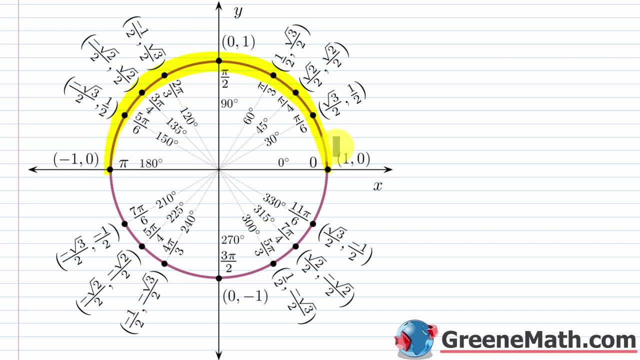 So now I'm looking here And if your argument is positive, you're going to look in quadrant one, And if it's negative, you're going to look in quadrant two. Again, there are exceptions to what I just said. Just like previously, if you have something like the inverse, 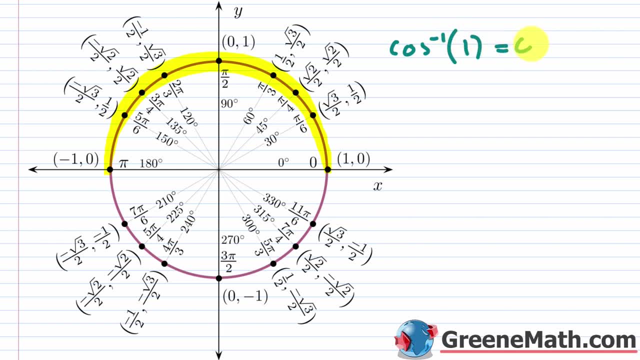 cosine of, let's say one. well, this is going to be zero, So that's going to be a quadrantal angle. If you have the inverse cosine of zero, that's going to be pi over two, So that's a quadrantal angle. 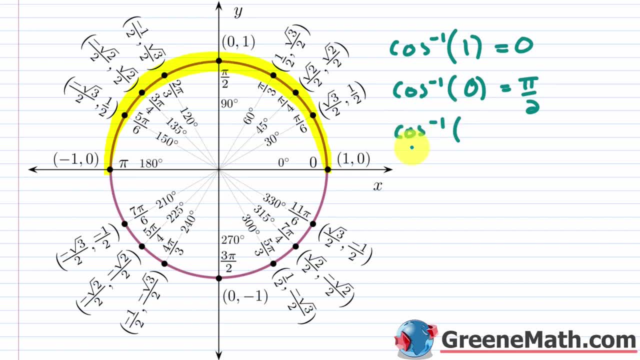 And then, lastly, if you had the inverse cosine of something like negative one, well, that's going to be pi. So basically, other than these guys, you can say that if your argument is positive, you're looking in quadrant one. 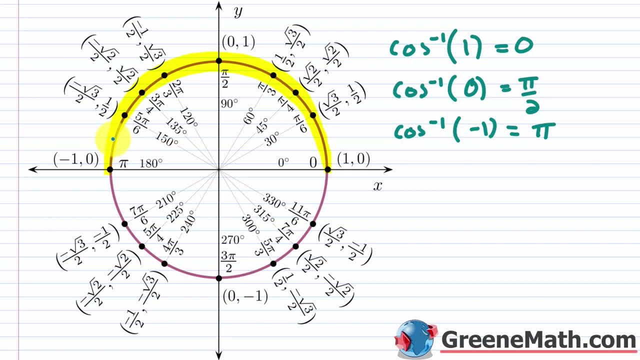 If your argument is negative, you're looking in quadrant two. The argument we have- let me get rid of this- is negative. So we're looking for the inverse cosine of the negative of the square root of three over two. So that tells me I want to look in quadrant two. 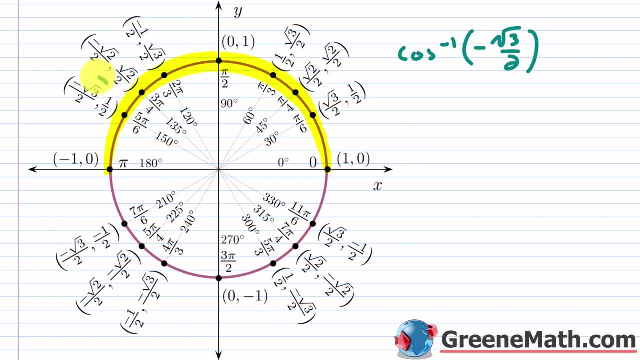 Looking in quadrant two, where cosine values are negative, I see that's going to occur right here. So there's my cosine value. I have negative square root of three over two And the angle that's associated with that is five pi over six. 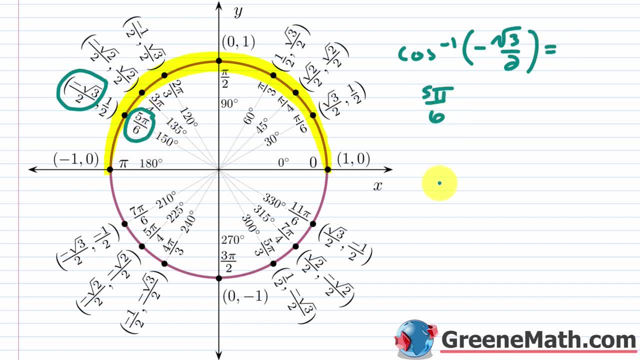 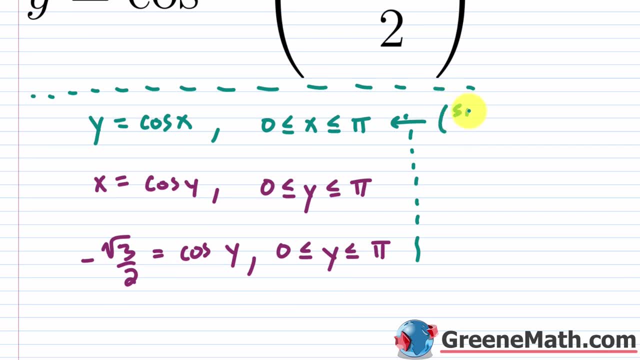 So the result here would be five pi over six. In other words, on the graph of this guy right here, the restricted cosine function, you have the point five pi over six, comma negative square root of three over two. So when you get to the inverse cosine function, these guys are going to be swapped. 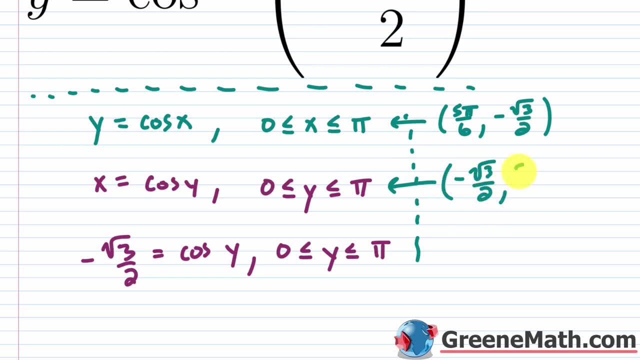 So you're going to have negative square root of three over two, comma five, pi over six. So when we answer this we basically just say that, And I think this is cut off too far. So let me just come down here and I'll just answer it formally. 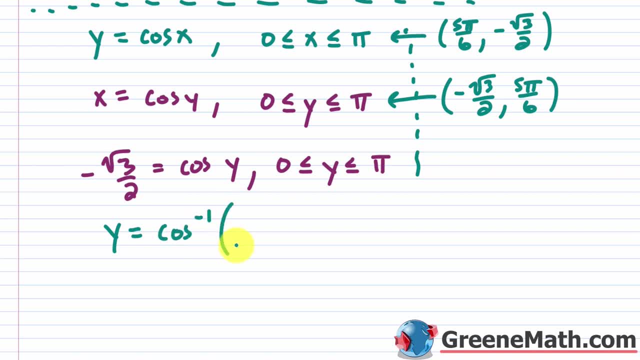 I will say that, if we have y is equal to the inverse cosine of the negative of the square root of three over two, that we're going to say that this is equal to five pi over six. All right, let's look at another one. 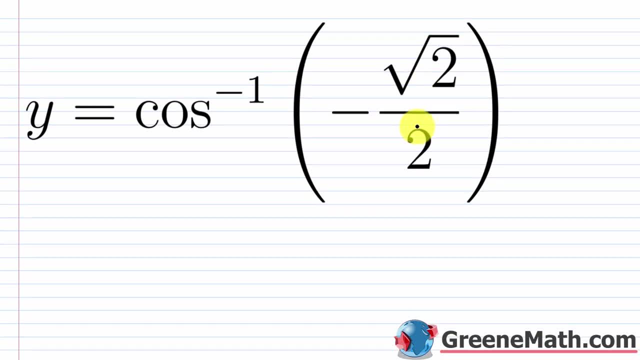 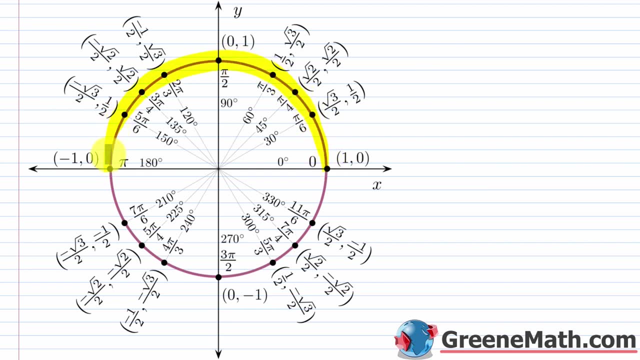 So we have: y equals the inverse cosine of negative square root of two over two. So again you can work off the unit circle. A lot of you know this off the top of your head, But we're working from zero to pi now, because that guy was a negative argument. 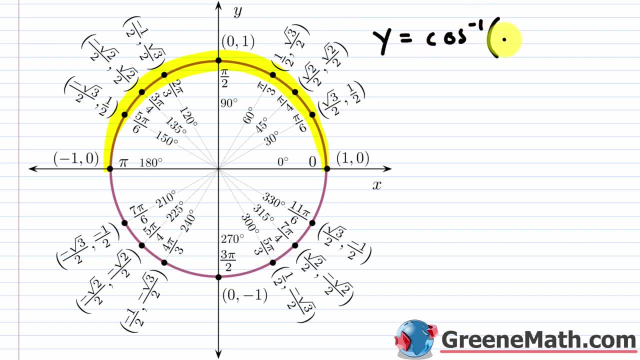 So in other words we had: y is equal to the inverse cosine of the negative of the square root of two over two. Again, when this guy is negative, I want to work in quadrant two. That's where cosine values are negative. So just find where you have a negative square root of two over two for the cosine. 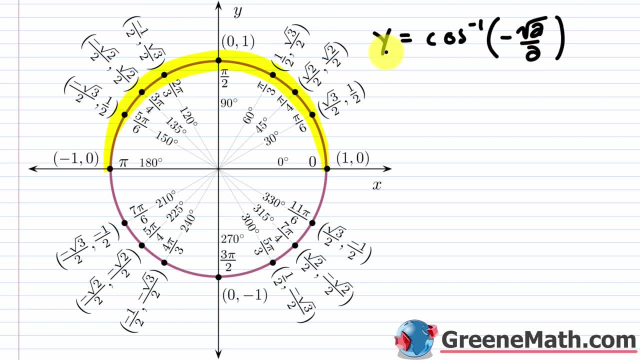 value and the y, there is going to be the associated angle. So basically I'm going to find that right here. Let me just highlight that. So you have a cosine value of a negative square root of two over two with your three, so with your three, pi over four. 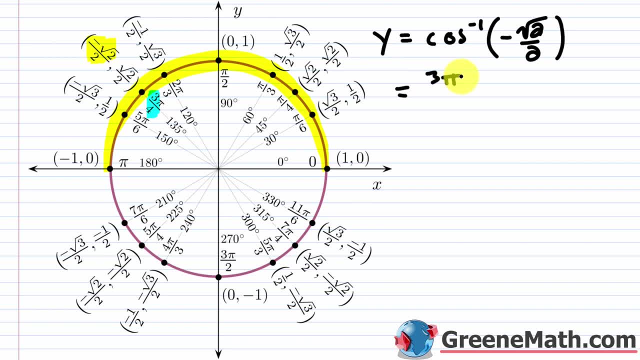 So the answer here for y is just going to be three pi over four Again, if you look at the restricted cosine function, so y equals the cosine of x, where x is greater than or equal to zero and less than or equal to pi. 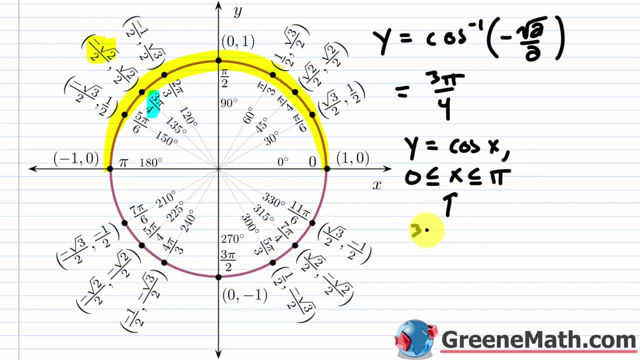 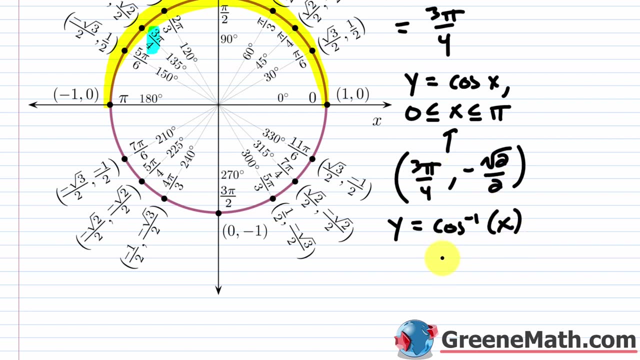 Well, a point on that graph is going to be three pi over four, comma, negative square root of two over two. So that's a point in the graph. So, when we think about the graph of the inverse cosine function, so y equals the inverse cosine of x- well, these x and y values are going to be swapped. 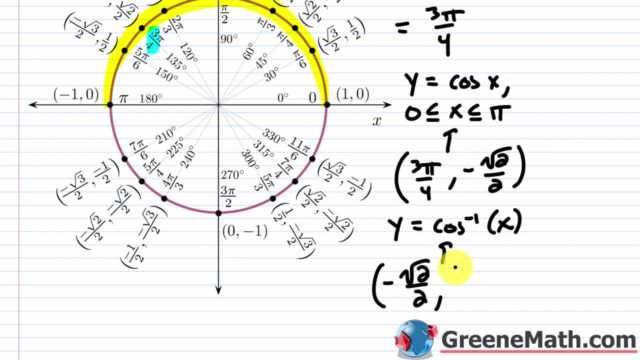 So now you have this negative square root of two over two and then comma three pi over four. So the inverse cosine of negative square root of two over two is going to give me three pi over four. All right, Just like with sine, you have the cancellation. 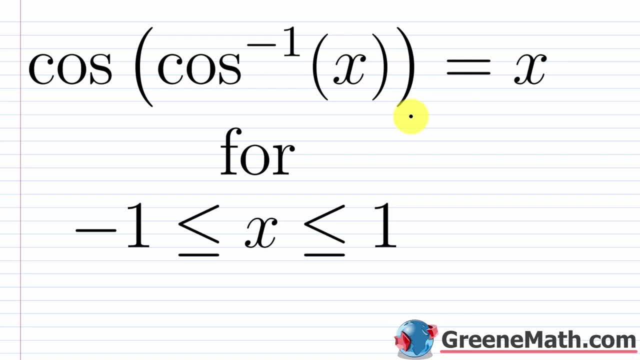 properties for cosine and the inverse cosine function when you put those guys together. So basically, if you have something like the cosine of the inverse cosine of x, it's equal to x, But only for x being greater than or equal to negative one and less than or equal to positive one. 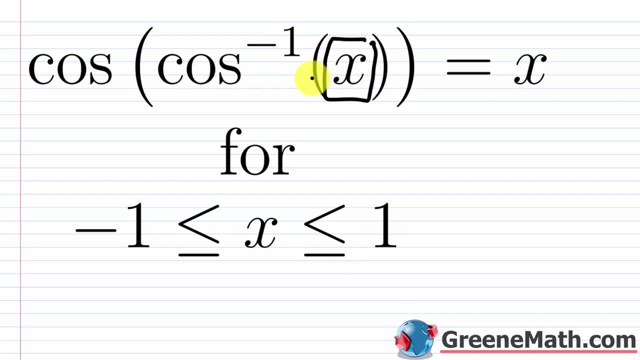 So the reason for that is, again, the domain for the inverse cosine function is going to be from negative one to positive one. You can't take something like the inverse cosine of two. Again, if you plug that into your calculator you're going to get some kind of error. 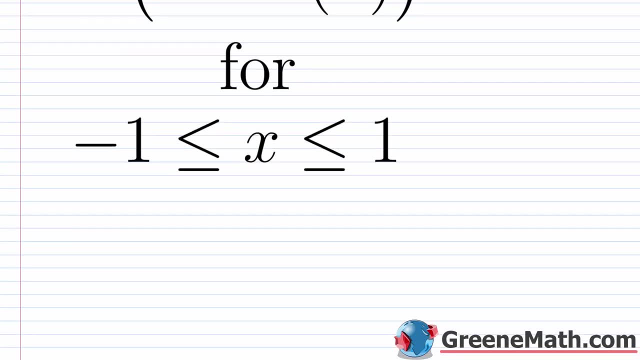 So what you would do. let's say we had something like- let me just slide down here real quick- the cosine of, let's say the inverse cosine of, let's say something like one half. Well, again, this right here would be in quadrant one. 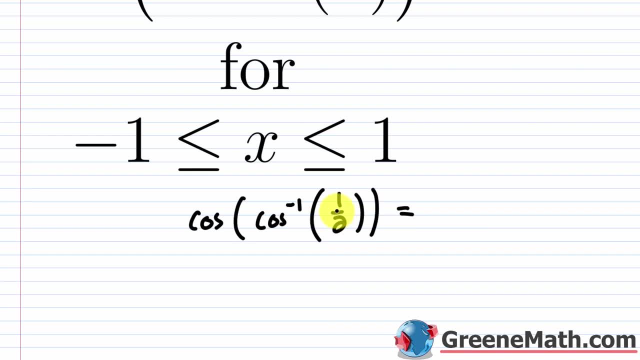 So I'm thinking about where is the cosine value? one half in quadrant one? Well, that's pi over three. So this, going the long way, would end up being the cosine of pi over three, And I'm right back to one half. So again, if this value satisfies this inequality, so it's greater than or equal. 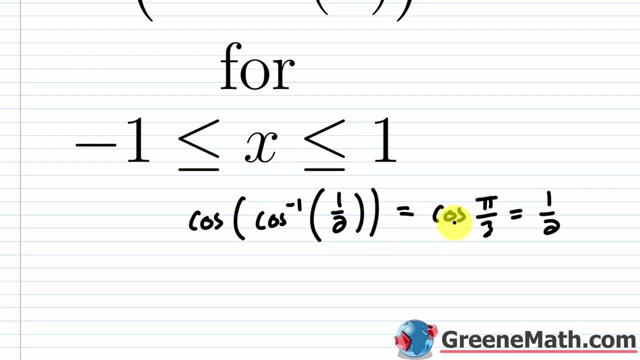 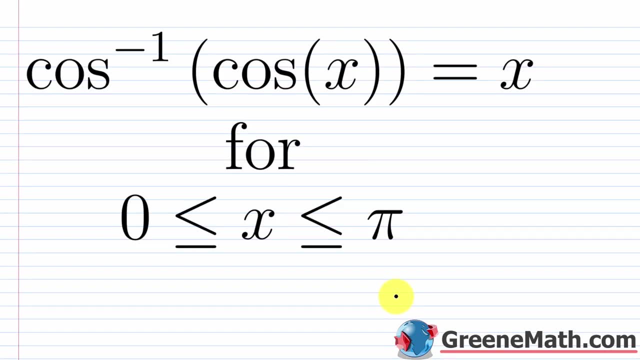 to negative one and less than or equal to positive one. you can just shortcut this process and immediately give the answer of one half, All right. So the other property involved is going to give you a lot of trouble if you're not paying attention. So the inverse cosine of the cosine of x. 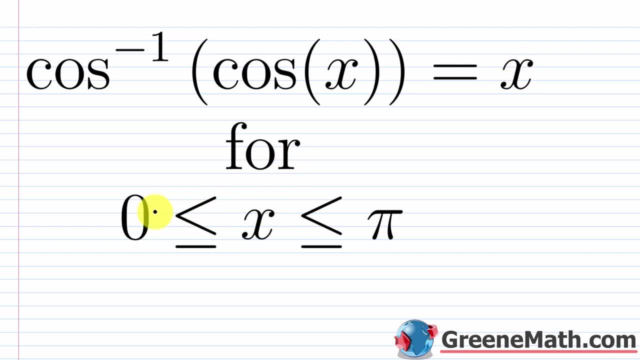 equals x. But this is the key. This is only for x being greater than or equal to zero and less than or equal to pi. Now, what's causing this? This is your regular cosine function on the inside, So we know that the domain is all real numbers. 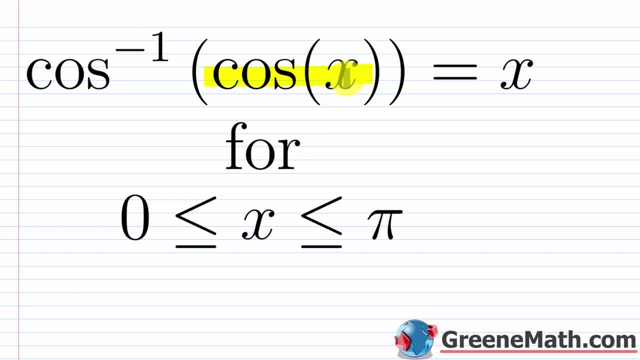 So really it doesn't matter what I plug in, for x Could be zero, could be negative, could be positive, It doesn't matter. We know that the range or the outputs here are going to be from negative one to positive one, and those guys are going to be included. 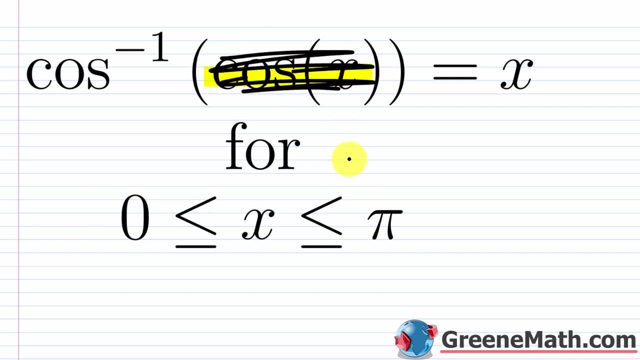 So let me actually just mark this out real quick so we can think about this. So I know that what I'm going to be plugging in here, for the inverse cosine function is going to be from negative one to positive one, And again, that is the domain of the inverse cosine function. 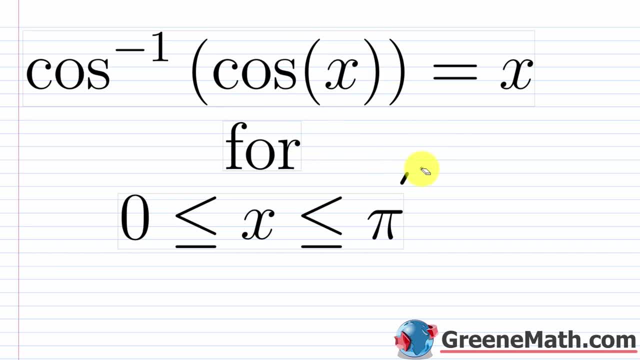 So I'm OK there. I'm never going to violate the domain, So let me erase this. And now let's think about this: When I take the inverse cosine of something from negative one to positive one, with those guys being included, I know that my range or my set of output. 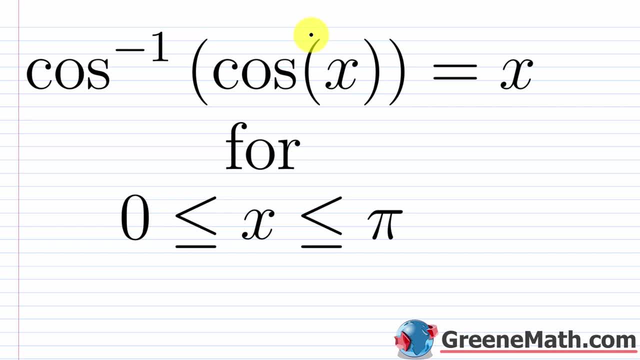 values is going to be from zero to pi, So that's why we have this, for x is greater than or equal to zero And less than or equal to pi. Now, if that was confusing, let me just give you an example here. 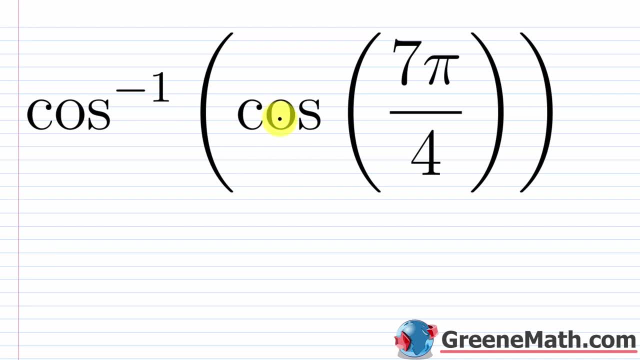 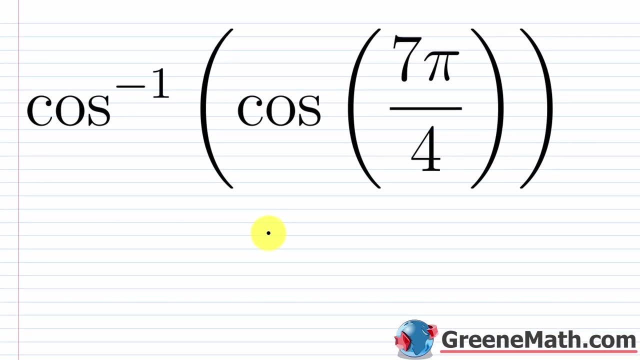 And hopefully this will make sense. So here we have the inverse cosine of the cosine of seven pi over four. Now seven pi over four is not in the interval from zero to pi, where zero is included and pi is also included If you go to the unit circle again. 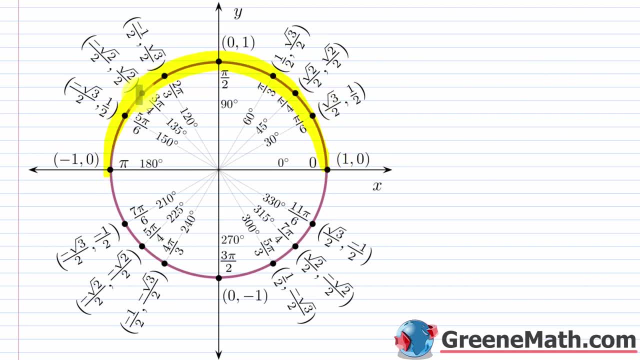 this is where we're working right here. So this is from zero to pi. Now, if we think about seven pi over four, that's down here, OK, so that's not in that interval. So what you'd have to do is say that you have the inverse cosine. 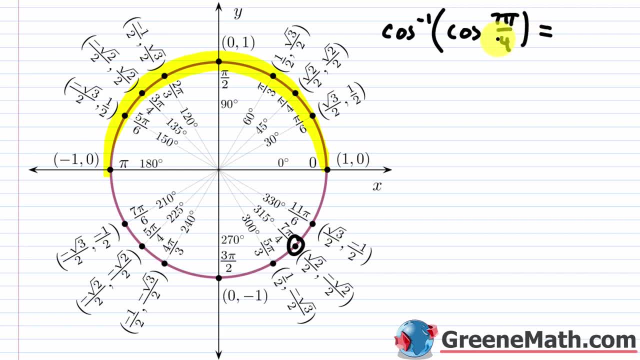 of the cosine of seven pi over four. You need to evaluate this first. So the cosine of seven pi over four, that's going to give you square root of two over two. So we're going to say this is the inverse cosine of the square root of two over two. 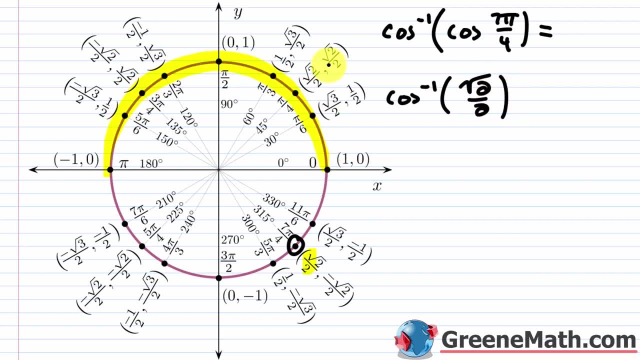 And again, looking at the correct interval here, you see where the cosine value is square root of two over two. That's going to be right here and that's going to be with pi over four. So you'd want to answer pi over four. 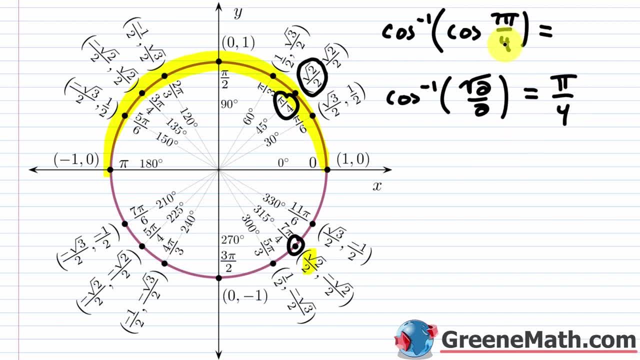 It is incorrect to say that the answer is seven pi over four, because that is not within the range of the inverse cosine function. So you have to be very, very careful with that type of problem. If you had gotten the problem- the inverse cosine- 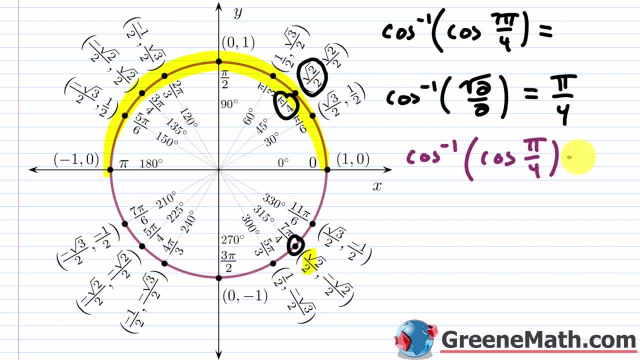 of, let's say, the cosine of pi over four. Well, in this particular case now you're within that interval, So these would just cancel away and you would say: this is pi over four Again. if you go through it the long way, which is fine, you can still do that. 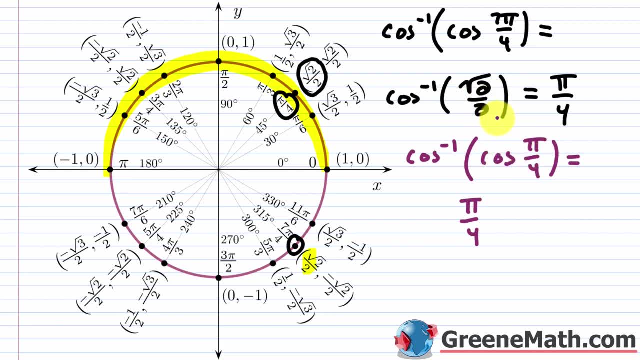 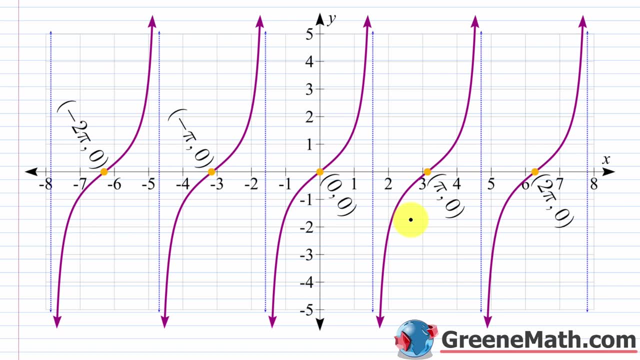 The cosine of pi over four, square root of two over two, And then the inverse cosine of square root of two over two, will get you back to pi over four. All right, Now let's talk about the inverse tangent function. So we're going to use the exact same. 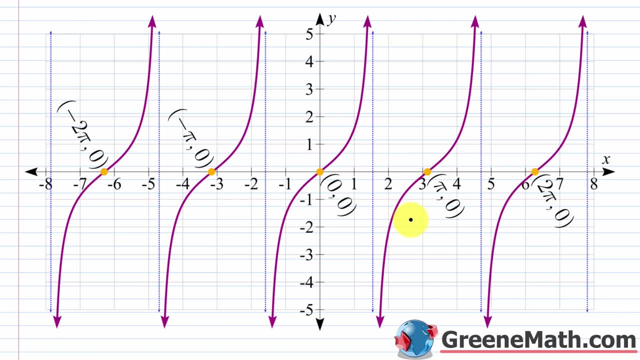 process that we used with the inverse sine function and the inverse cosine function. So we're going to start off with a graph that we already know about. So that is, y is equal to the tangent of x. Now, when you graph this guy- hopefully you've seen this already- 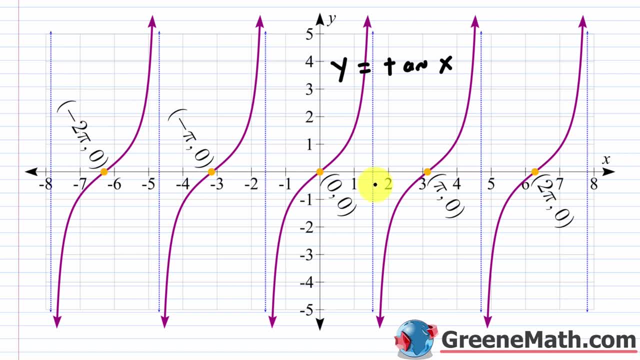 You know that you have a series of vertical asymptotes and that's going to be at odd multiples of pi over two. So something like this is at pi over two, And then this guy right here is going to be three pi over two, And this guy right here is going to be five pi over two. 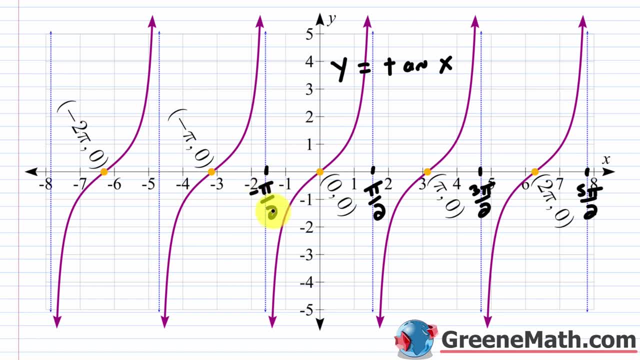 And if you were going this way, so this right here would be negative pi over two, And then this right here would be negative three pi over two, And then this guy right here would be negative five pi over two. So again, what causes that? 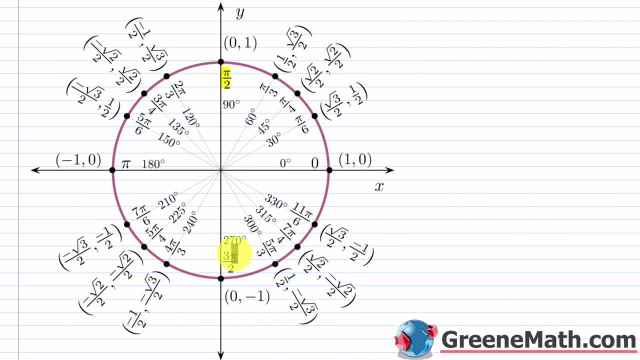 Well, if you go back to the unit circle, if you look at something like pi over two or three pi over two, the cosine value is zero, And this is going to be true for pi over two, three pi over two, five, pi over two. 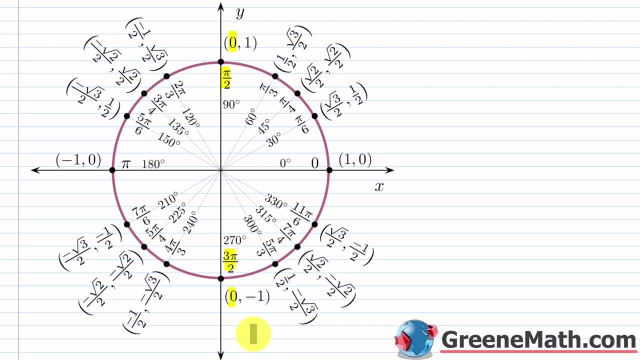 seven, pi over two, so on and so forth. So a lot of books will just say odd multiples of pi over two. So what happens is when you look for the tangent of something like that, if the cosine value is zero you have the sine value divided by the cosine value. 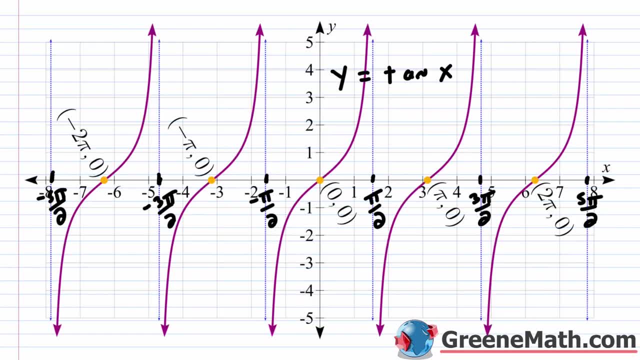 And again, if you're trying to divide by zero, that's undefined. So, coming back up, that's why you see these vertical asymptotes here. So for the domain, so for the domain, and I'm going to write this in set builder notation. 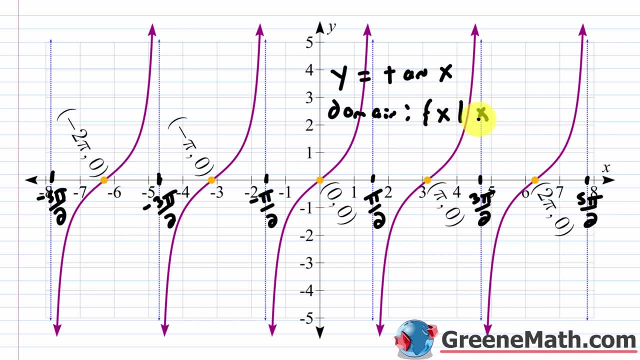 So I'm going to say that it's the set of all X, such that X is not equal to. We're going to start with pi over two and then just say plus pi n, And here, specifically, n is just going to be any integer. 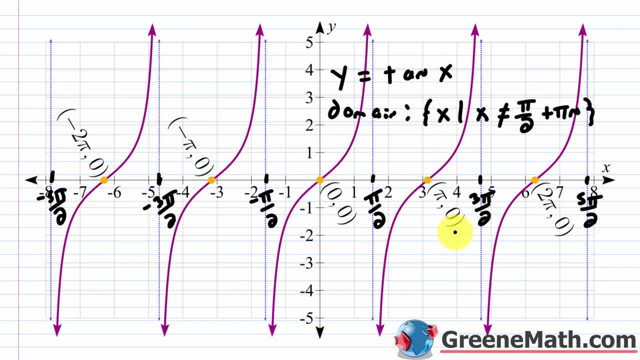 So if you added pi to pi over two, you would get three pi over two. Then if you added, let's say, two pi to pi over two, you would have five pi over two, so on and so forth. Now, in terms of the range, there's no restriction, right. 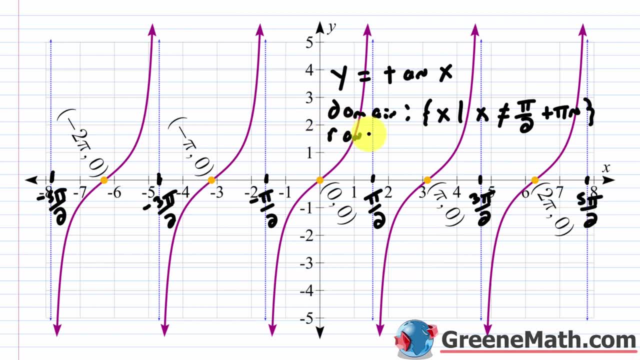 So this is from negative infinity to positive infinity. So for the range we're going to go, I'll just use interval notation, It's a little bit easier. So from negative infinity to positive infinity, So basically all real numbers. Now, when we look at the graph of Y equals the tangent of X, obviously. 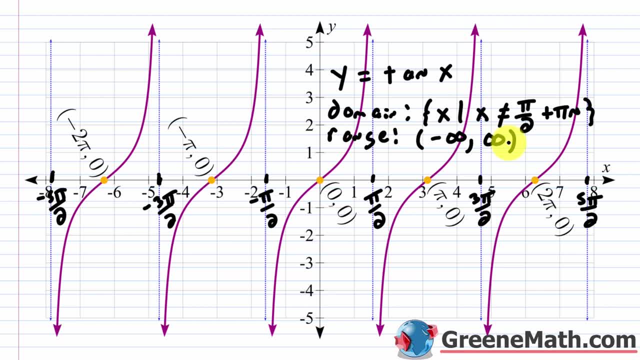 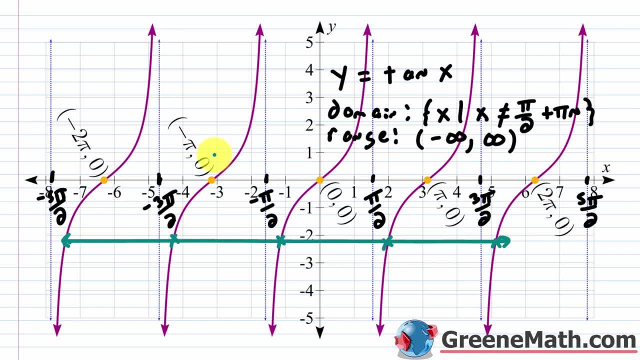 So it's going to hit over and over and over again. So obviously, this is not the graph of a one to one function. So what do we do? Well, just like before, we're just going to take a piece of this graph such that we have a restricted 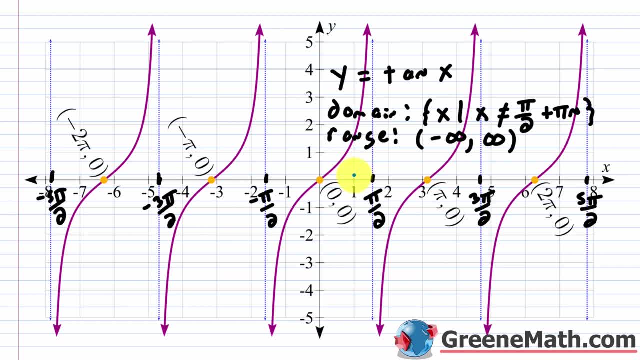 line, but we keep the same range. So what we've chosen to do in this situation is go from negative pi over two to pi over two, with those values being excluded because, again, tangent of negative pi over two or tangent of pi over two, that's undefined because you'd have division by zero. 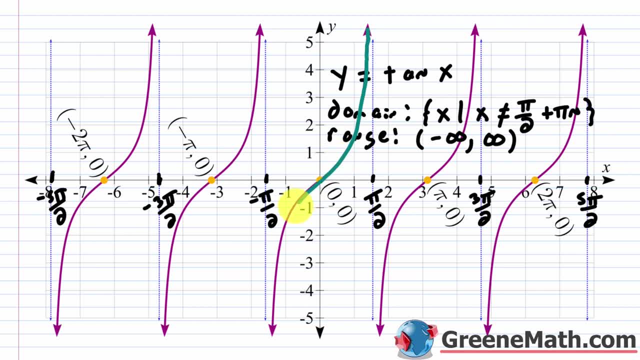 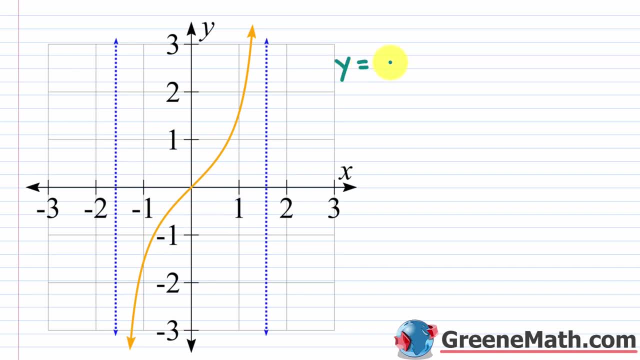 So this is the piece that we're going to take right here. So that's what we're looking for, And let me just show you that using a better graph. So this right here would be: your Y is equal to the tangent of X, where X. 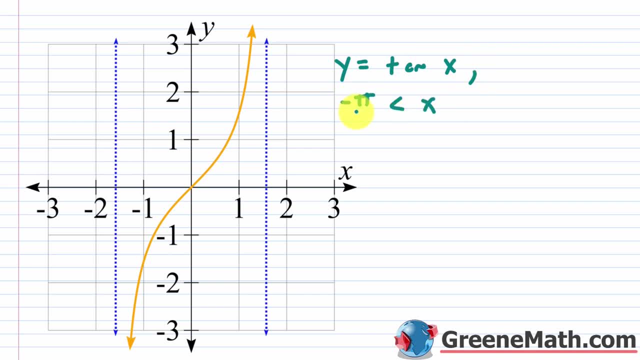 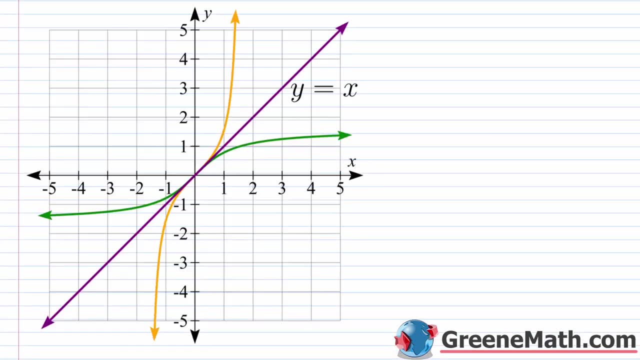 is greater than- and this is strictly greater than negative- pi over two and less than- and that's strictly less than- pi over two. So this is your restricted tangent function And, just like before, if you reflect that across the line Y equals X, you'll get your inverse tangent function. 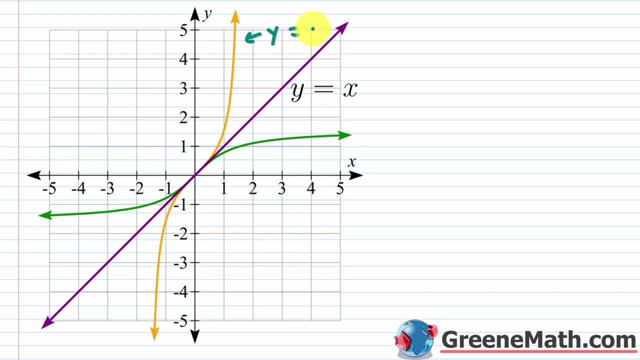 So this right here in orange- this is your Y- equals again the tangent of X, where X is greater than negative, pi over two and less than pi over two. And then the graph in green Here this is going to be: your Y is equal to the inverse tangent. 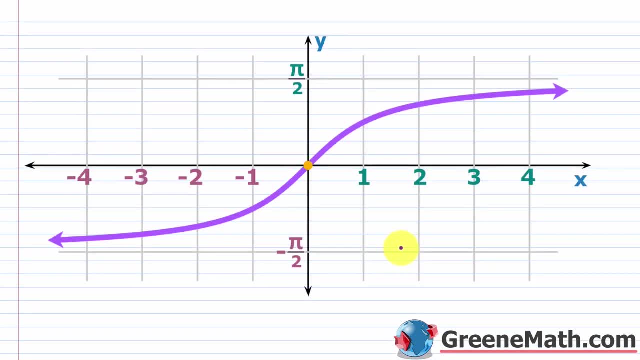 So the inverse tangent of X. So let's go down to this little graph here where things are easier to see. So let's write that this is Y equals the inverse tangent of X, And for the domain, you'll see that it's the set of real numbers. 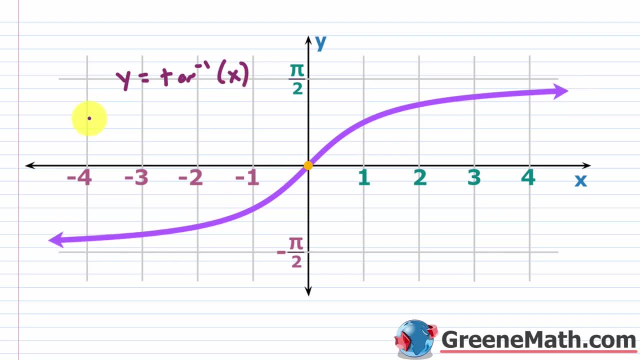 So I can plug in whatever I want for X. there There's no problems. So I'm going to say that my domain is just going to be from negative infinity to positive infinity. And if we think about where that comes from, well, think about the range. 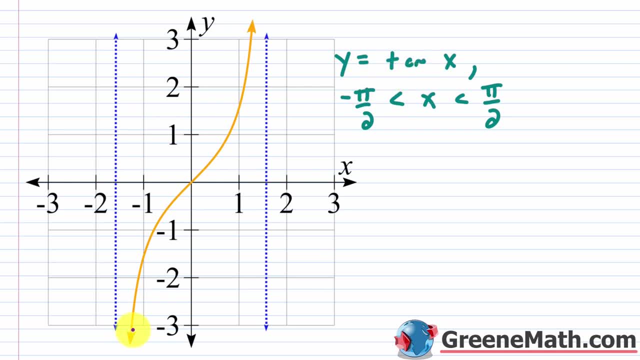 of the restricted tangent function is from negative infinity to positive infinity. So when we get the inverse, the domain becomes the range and the range becomes the domain. So this range here from negative infinity to positive infinity became the domain here of negative infinity to positive infinity. 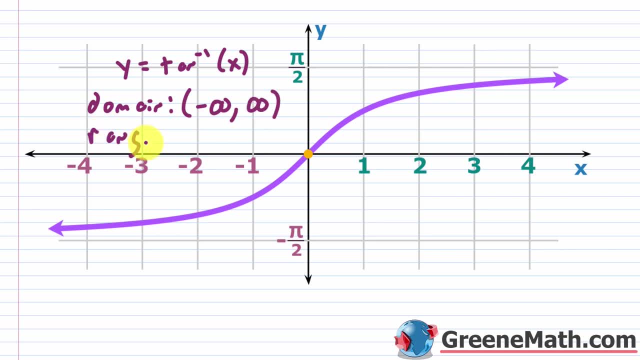 Now, similarly, when we look at the range here, This is coming from the domain of the restricted tangent function, which was from negative pi over two to pi over two, with those guys being excluded. So this is really important. You want a parenthesis here for negative pi over two. 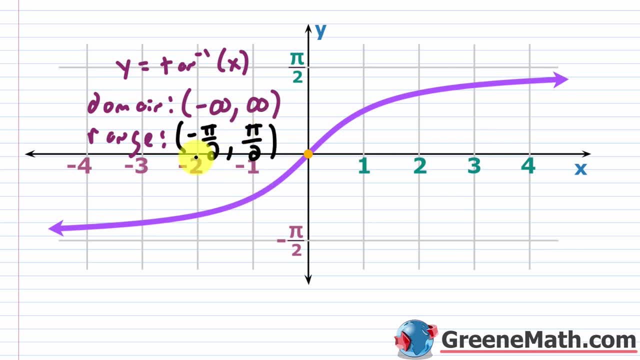 It's not included, And then a parenthesis next to pi over two because it's not included. So this value up here and this value down here, they're not included. So you'd have a horizontal asymptote here and also here. So these graphs will approach those values but never actually touch them. 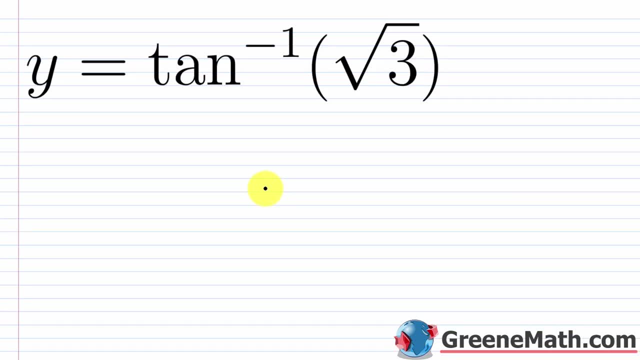 OK, let's take a look at some problems. So we have: Y equals the inverse tangent of square root of three. So again, when I look at something like this, I always go: Y is equal to the tangent of X And I'm going to say: X is greater than negative pi over two and less than pi over two. 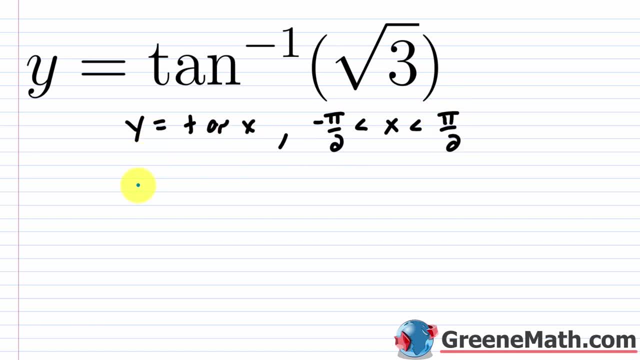 And again I'm just going to swap X and Y to find the inverse. I'm going to say X is equal to the tangent of Y where specifically, again, this was the domain. So now it becomes the range. So Y is greater than negative, pi over two and less than pi over two. 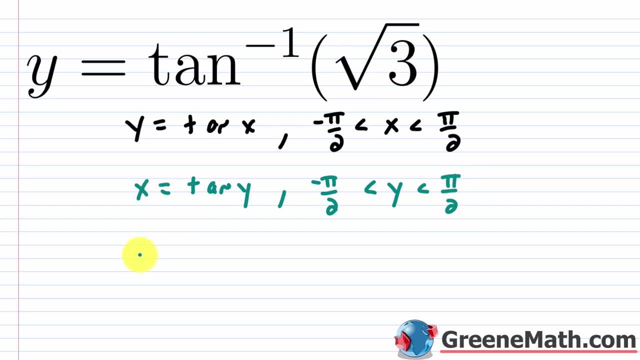 So if I plug in a square root of three for X there, so we'd say the square root of three is equal to the tangent of Y, And again, where Y is greater than negative, pi over two and less than pi over two. Well, let's think about this for a moment. 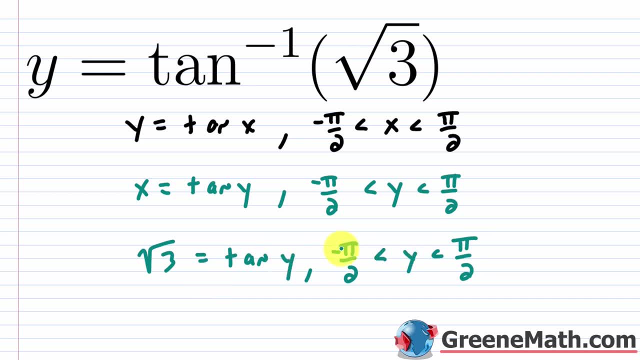 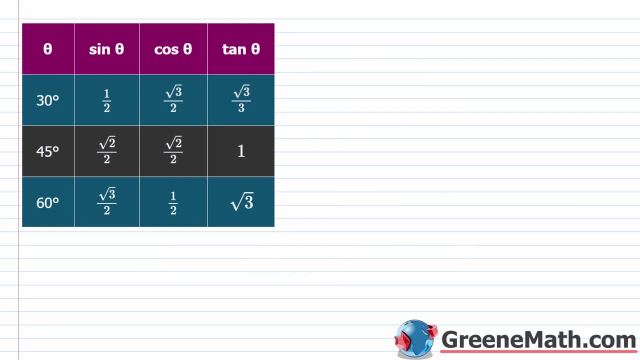 I'm asking for the angle in the interval from negative pi over two to pi over two, such that the tangent value is going to be the square root of three. Well, you can use special triangles. We'll go to the unit circle in a moment. 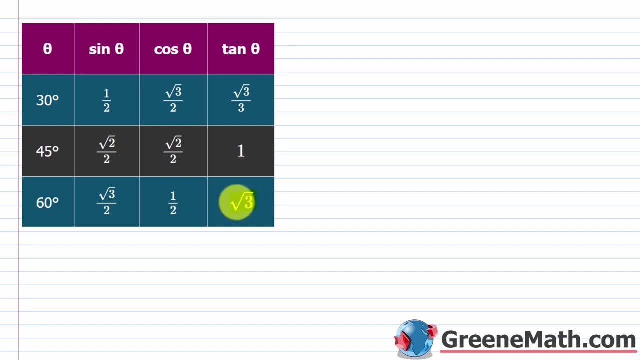 If you look at a tangent value of square root of three, so that's going to be right there. I don't think my highlighter really shows up there, So maybe I can use a different color like black. I think that might show up a little bit better. 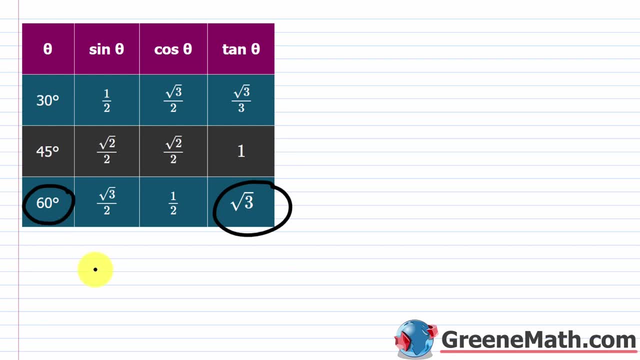 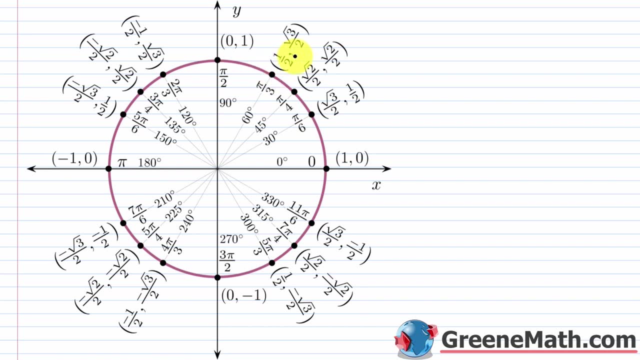 So basically you can see that's going to happen at 60 degrees. Or if you want to convert this into radians, that's going to be pi over three. Additionally, you can always go to the unit circle and use that. The values aren't directly there. 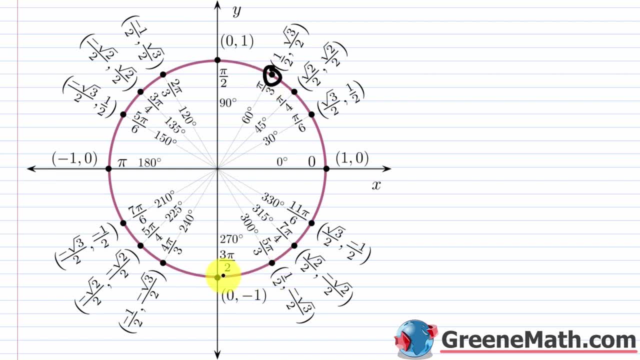 But if you look at pi over three again, that's in your interval, You're working from negative pi over two to pi over two. The key thing is here that pi over two and negative pi over two are not included. Okay, So it's not like sine, where they are included. 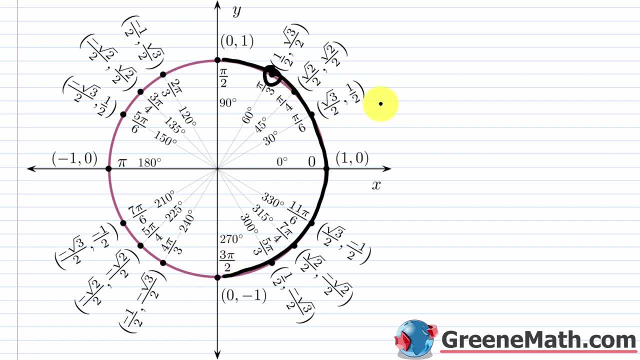 Here they're excluded. So if I look at that, that's within the interval. And again, if you look at the tangent of pi over three, well, really quickly you can just look at: well, it's the sine of pi over three. 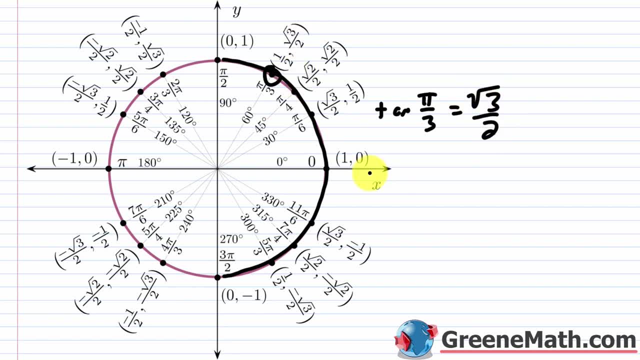 which is the square root of three over two, divided by the cosine of pi over three, which is basically going to be one half. So times the reciprocal, which is two over one, Those twos cancel and you get the square root of three. 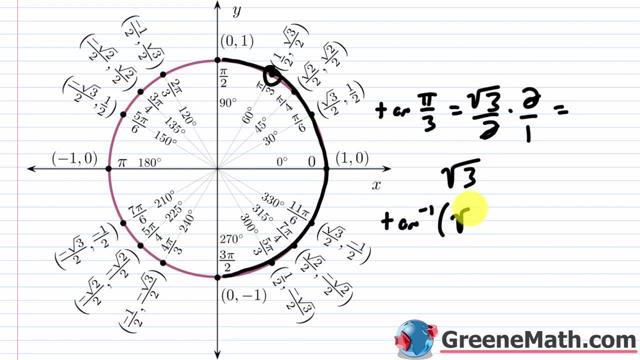 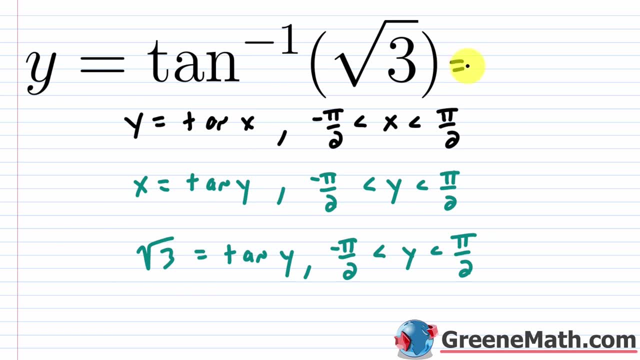 So that tells me that the inverse tangent, So the inverse tangent of the square root of three, is going to be pi over three, because again it's in this interval. So let's come back And I'm just going to answer that this guy right here is going to be pi over three. 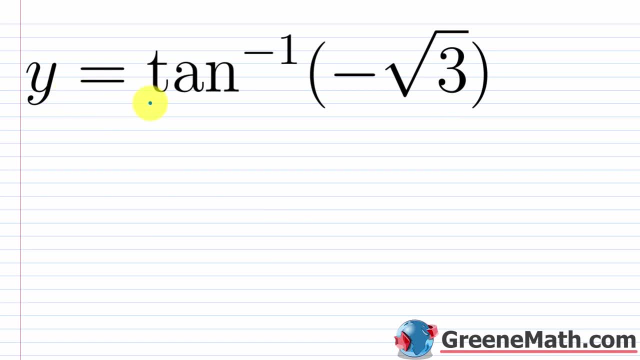 Okay, Let's look at another one, So this will be real easy. We have: y equals the inverse tangent of the negative of the square root of three. So, first off, what you could do to solve this problem. the inverse tangent function and the inverse sine function are odd functions. 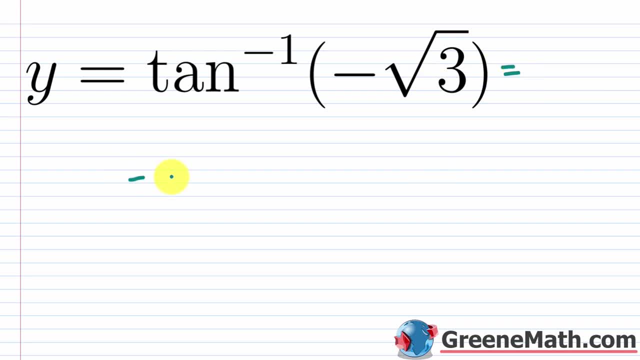 So you could say that this is equal to the negative of the inverse tangent of the square root of three. And we saw earlier that the inverse tangent of the square root of three was pi over three. So this would be the negative of pi over three or just negative pi over three. 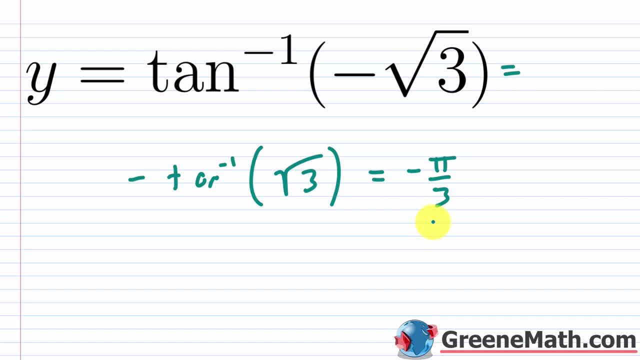 So that's the quickest way to solve that, given the fact that you know that the inverse tangent of square root of three is pi over three. Now the other way: let's just do this the longer way, just so we can see it. 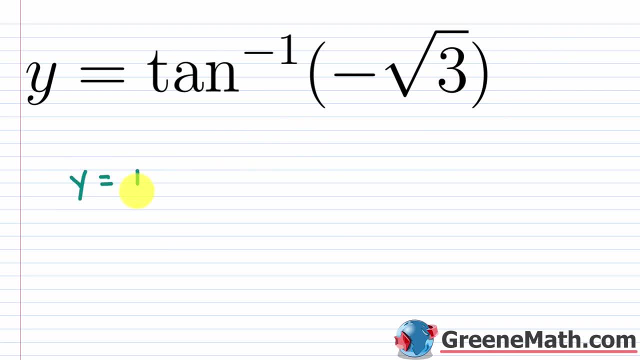 The first thing is, if I know that y is equal to the inverse tangent of the square root of three is going to be equal to pi over three. We already know that. Well then, what I can do is go to my unit circle and look for an angle in quadrant. 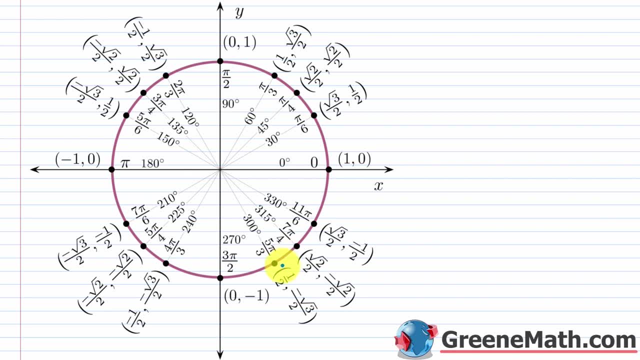 four, where tangent is negative and I'm going to want a pi over three reference angle. So here I'm going to rotate clockwise to get to right there. So this is not going to be five pi over three, It's going to be negative pi over three. 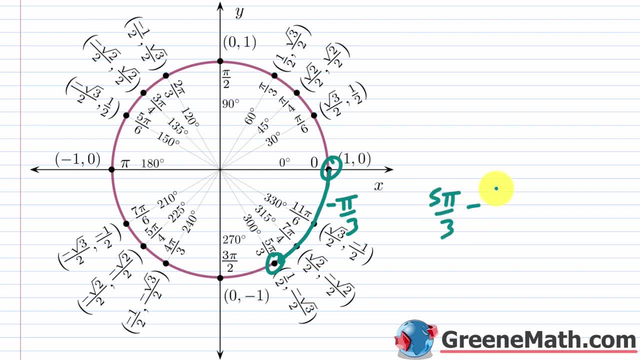 Again, you can start with five pi over three if you want, and just subtract away two pi so that six pi over three and you can get the negative pi over three, like that, if you want. Again, it's up to you how you want to do things. 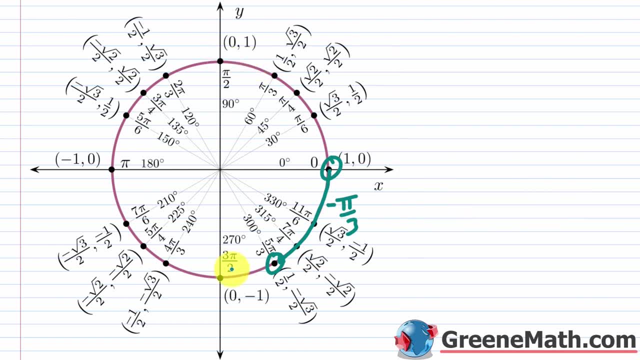 But essentially you want to make sure that you're in that interval again from negative pi over two to pi over two. Let me highlight that real quick. So I'm going to make sure to not touch pi over two or negative pi over two. 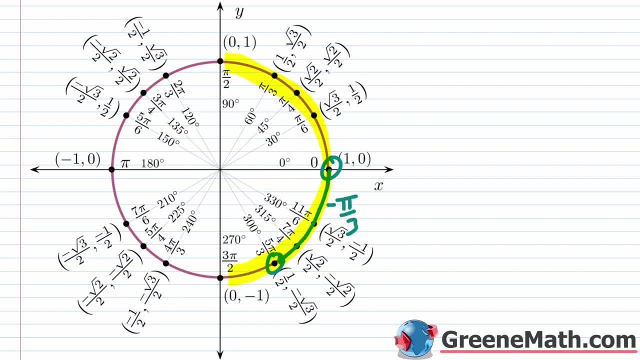 Those are not included. So as long as you're in this interval, you're going to be good to go. So, basically, because the tangent of negative pi over three is equal to the negative of the square root of three, Well, because again this is in that interval, you can say that the inverse 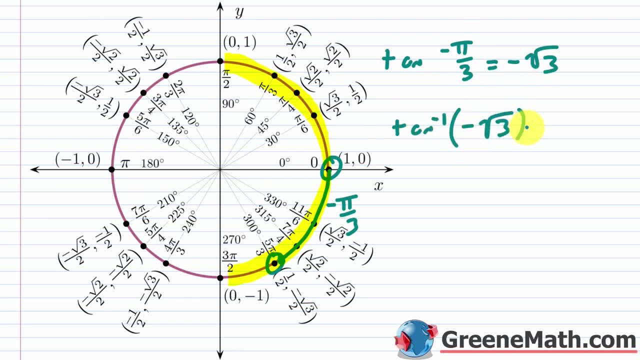 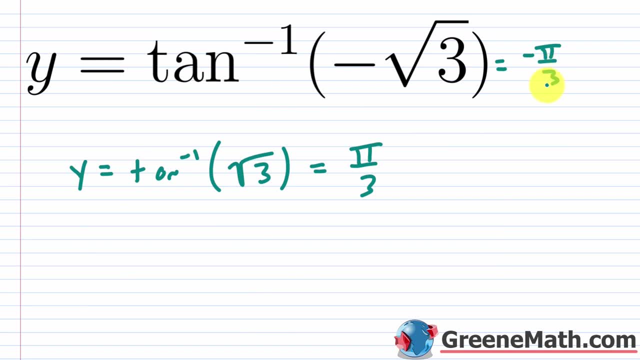 tangent, so the inverse tangent of the negative of the square root of three. that's going to be negative pi over three. So, coming back up, the answer here once again is negative pi over three. All right, let's look at some cancellation. 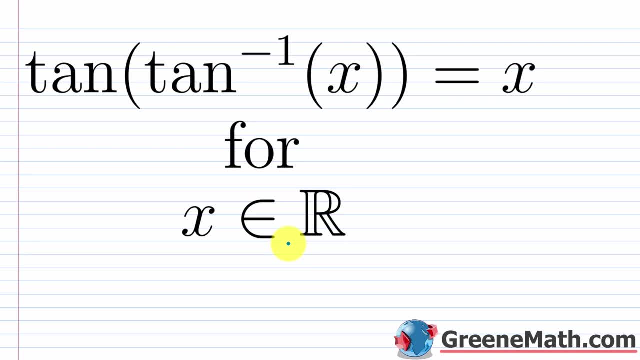 properties with tangent and inverse tangent. So these are very similar to what we saw earlier. So the tangent of the inverse tangent of X is equal to X for any X. That's a real number. So that's basically what this is saying. This says X is an element of the real numbers. 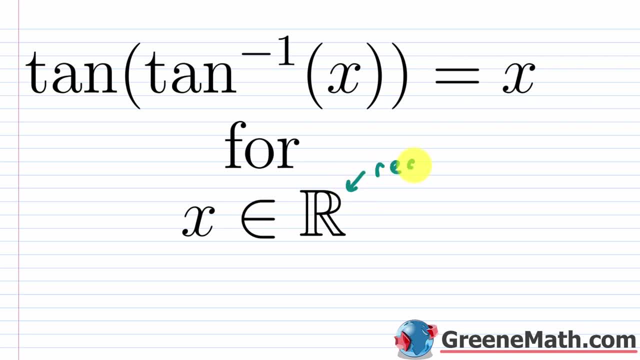 Whenever you see this R that looks like this, this means the set of real numbers, So let me write that out. So the set of real numbers- and this right here, if you've never taken a course on sets, this just means is an element of 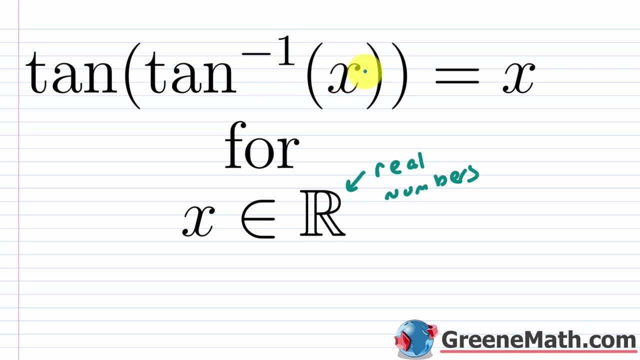 Now when we think about the inverse tangent function, remember the domain is the set of real numbers, So I can plug in whatever I want there for X and the output will be between negative pi over two and pi over two, with those values being excluded. 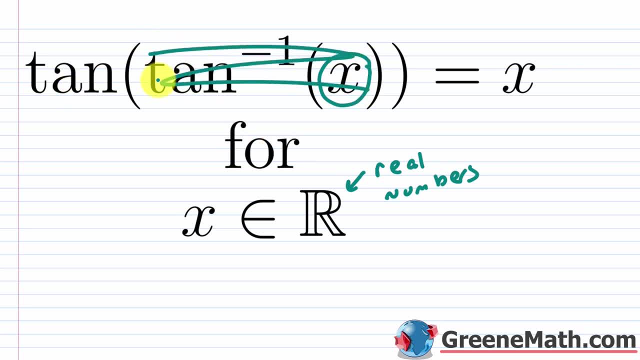 So that means again, you could just mark this out and say: OK, well, the tangent of between negative pi over two and pi over two, that's always going to be defined, so I won't really have any issues there. So I can just basically cancel things away and say that I just have X. 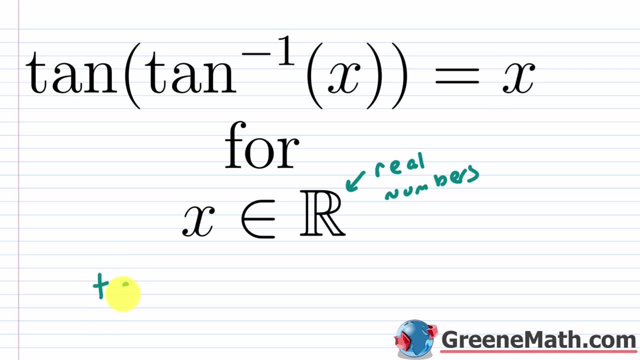 So if you wanted to see an example of that, you could just quickly do something like the tangent of: let's say, the inverse tangent of: let's just go ahead and do something like: maybe the square root of three over three, something like that. 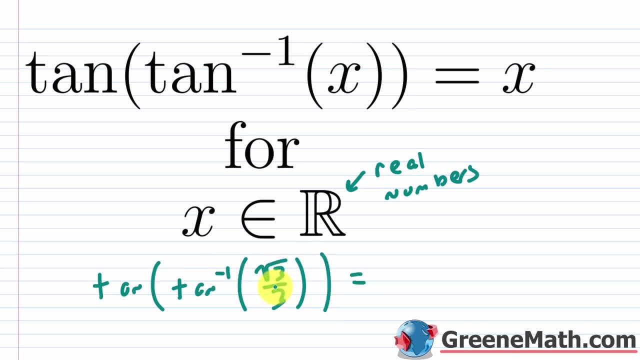 I think most of you know that the inverse tangent of the square root of three over three is going to be pi over six. So this would be the tangent of pi over six. And again, the tangent of pi over six is going to get me back to the square root of three over three. 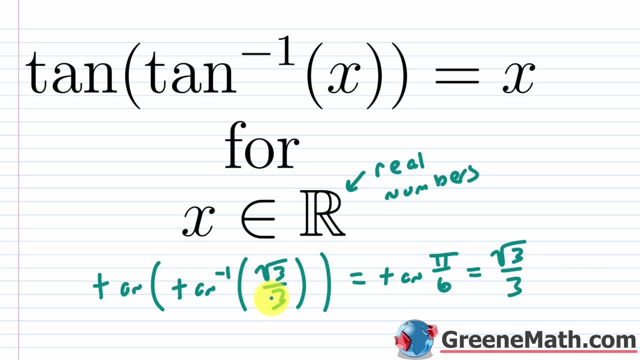 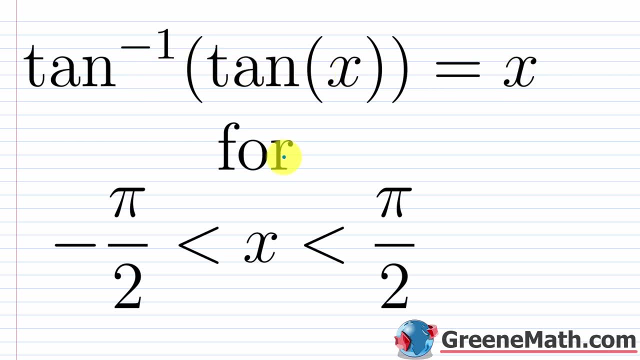 So you could have just shortcutted the process and just said the answer is square over three. All right, let's look at the other one, And this one is where people get into trouble. So the inverse tangent of tangent of X is equal to X, for X is greater than negative pi over two and less than pi over two. 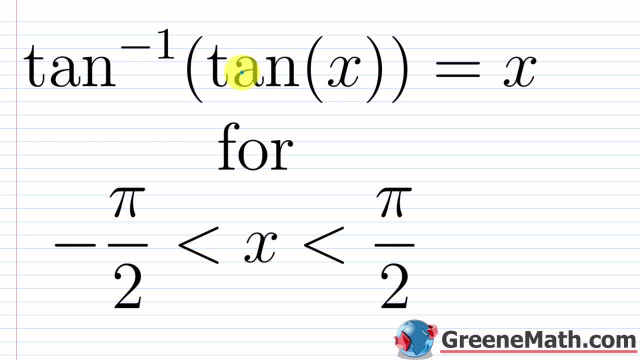 So let me walk you through this one. So basically, let's start off with the tangent of X, So the inside part here. we know that for this guy right here X cannot be pi over two, three pi over two, five, pi over two. 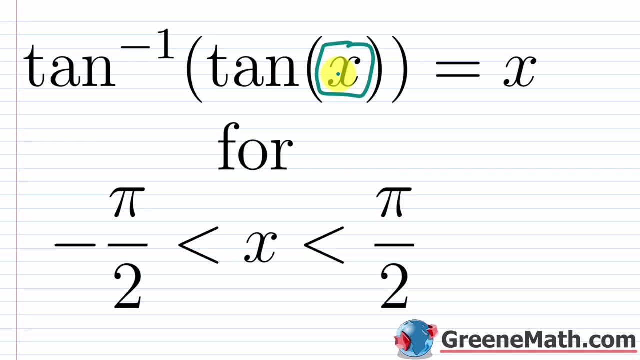 So you could say pi over two plus pi n where n is an integer. or you could say something like odd multiples of pi over two. whatever you want to do, But basically assuming that this guy right here, you don't plug in something that gives you undefined as a result. 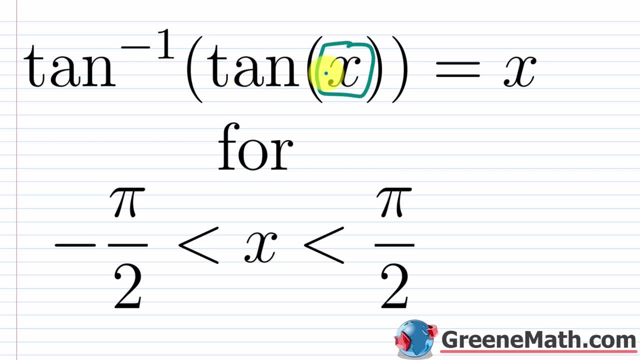 Well then we know that the range for the tangent of X is going to be all real numbers. So, assuming that you didn't plug in something that violated the domain to where you got undefined, the result of this guy right here would be all real numbers. 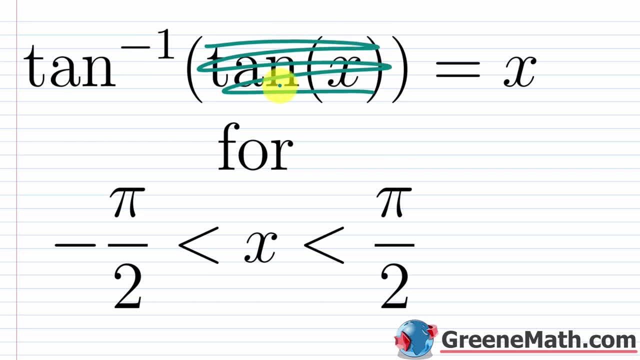 Now when you take the inverse tangent again, the domain is all real numbers And when you plug in all real numbers for this guy, you're going to get basically between negative pi over two and pi over two as a result. So that's why we say this is for X is greater than negative pi over two and less. 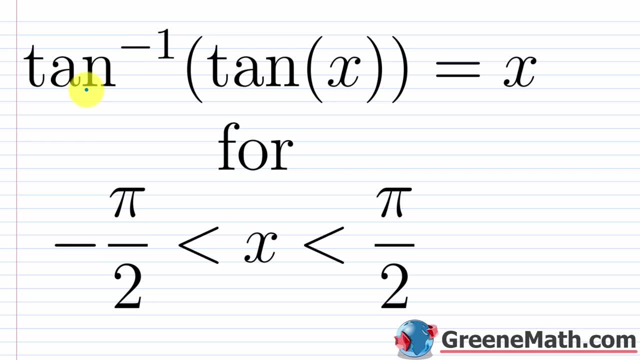 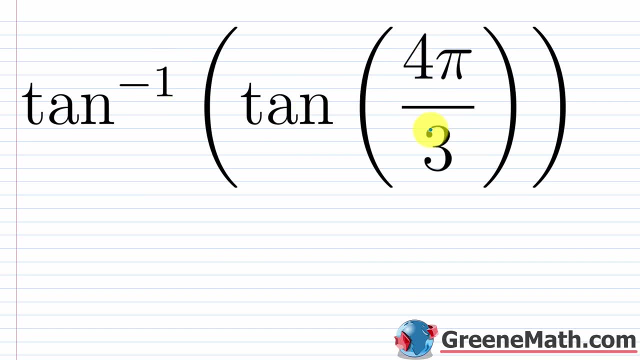 than pi over two, because again that's from the range of the inverse tangent function. So let's look at an example. So here we have the inverse tangent of the tangent of four pi over three, So the tangent of four pi over three, that's defined. 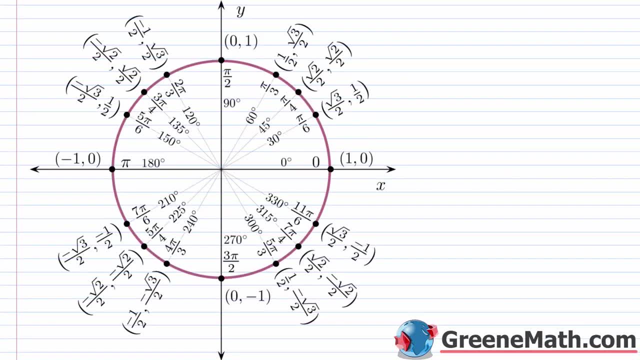 But it's not within that range from negative pi over two to pi over two. So coming back to the unit circle again, thinking about from pi over two to negative pi over two, Again those guys are excluded. So I'm trying to stop short. 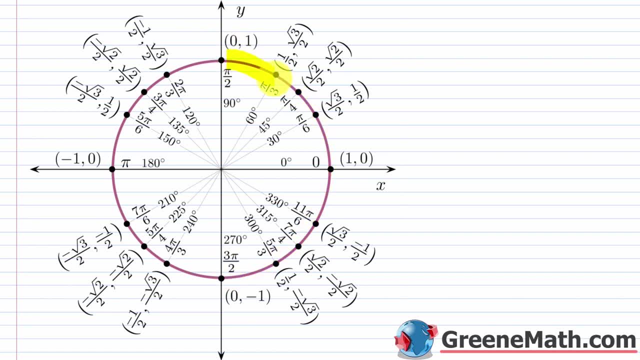 I'm trying to make sure that I'm not missing anything there And maybe I touched there, So let me try this one more time. I want to make that crystal clear that pi over two and negative pi over two are not included. So you're looking at this angle right here, which is four pi over three. 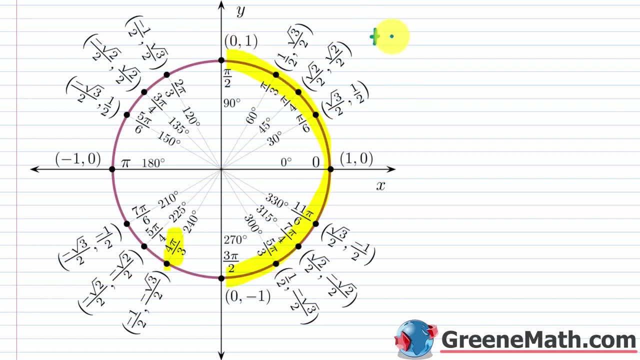 So that's not in that interval. So what you would have to do is first say that I want the tangent of four pi over three. Now, this has a pi over three reference angle and you're in quadrant three. So we know that this would be equal to the tangent. 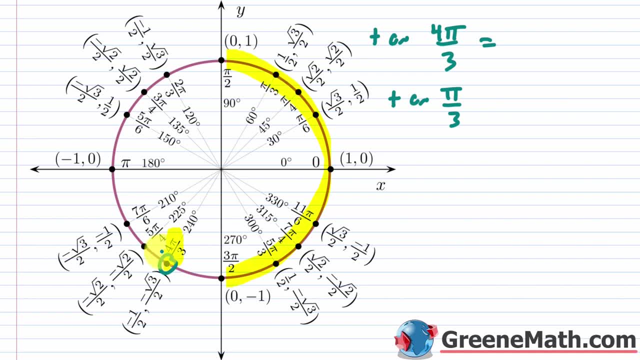 of pi over three. So the tangent values are positive in quadrants one and three. So essentially, if I look at this guy right here, the tangent of pi over three it's going to be the same as the tangent of four pi over three. 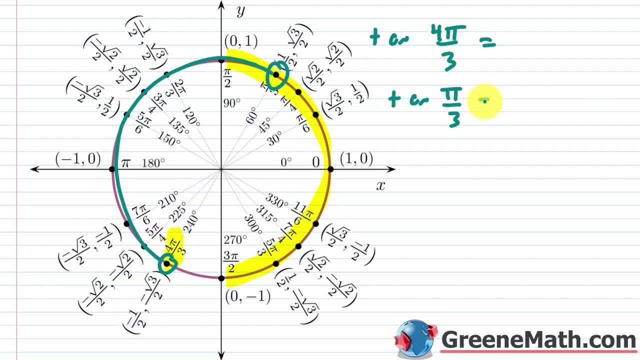 Again, the period for tangent is going to be pi, So the tangent value is going to be the same there. So this is going to be equal to, as we saw earlier, the square root of three. So essentially, when we solve this problem, 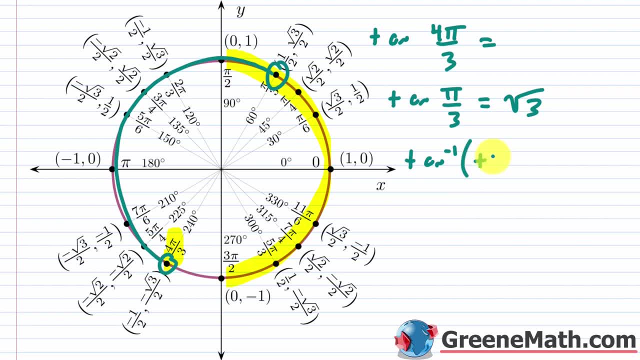 if we say something like the inverse tangent of the tangent of four pi over three, what you need to do is the tangent of four pi over three. So this is the inverse tangent of. again, that would be square root of three. So square root of three, And then this equals what? 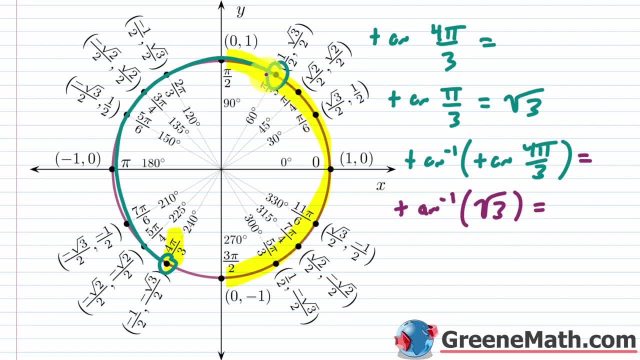 Well, where is the tangent value square root of three in this interval here? Well, it's going to be at pi over three. So that puts me right back to pi over three. So you've got to be really careful with these types of problems. 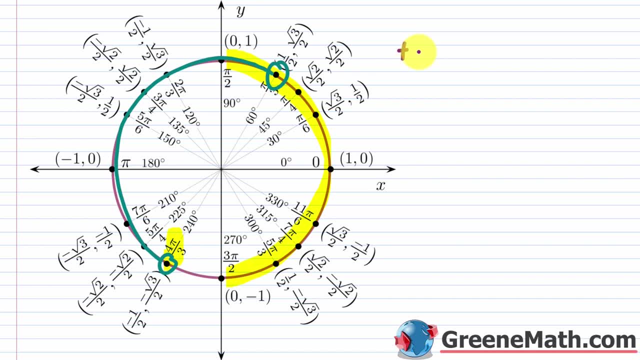 Now again, if you had gotten the problem as something like, let's say, the inverse tangent of, and let's go tangent of negative pi over three. We saw that earlier. Well, this guy right here is in your interval, so we know that that's going. 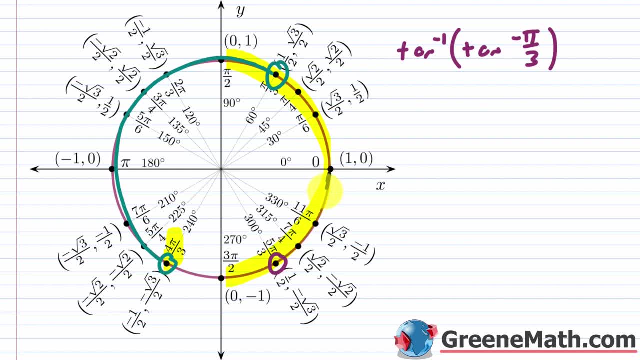 to be right here again rotating- Let me do this in a different color- So rotating clockwise, like that. So that's my negative pi over three. So I can just take that in this case That'll be the answer. So this is just negative pi over three. 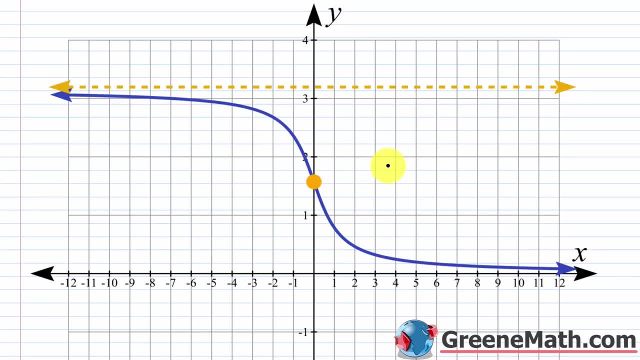 All right, Now let's look at some problems that deal with the inverse cotangent function, the inverse secant function and the inverse cosecant function. So these problems are pretty easy If you already understand the inverse sine function, the inverse cosine function and the inverse tangent function. 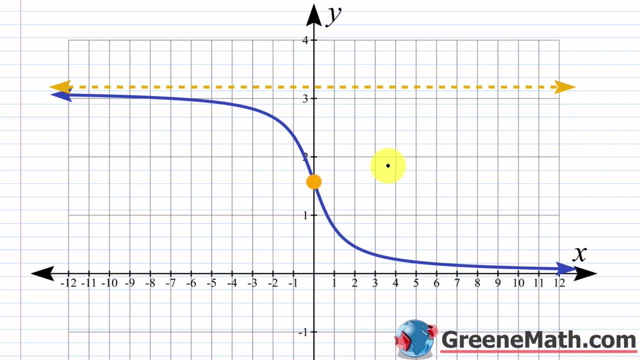 you can actually convert them over and use those guys to get your solution. So let me start with: y is equal to the inverse cotangent- Let me make that a little bit cleaner there- of x. If you're looking this up online or if you're using a textbook, that's different. 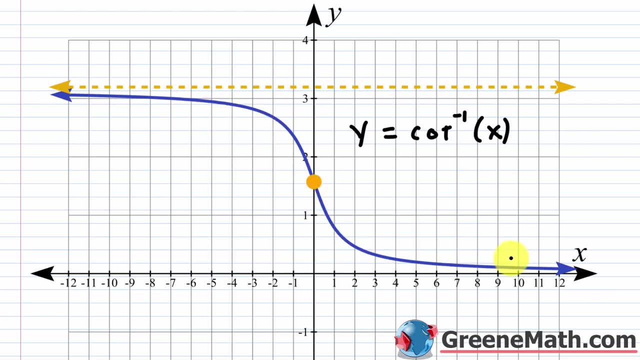 from mine, you might see a different graph, And the reason for that is very simple. When you derive this guy, you start off with: y equals the cotangent of x. So we know that that guy right. there is not a one to one function. 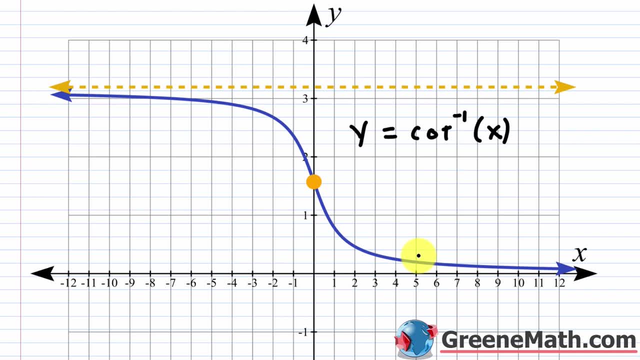 We also know it's not defined for pi, n or n as any integer, because if you have something like zero or pi, or two pi or three pi, your sine value is going to be zero and you'd have division by zero, which is undefined. So what you could do is take a piece of that guy. 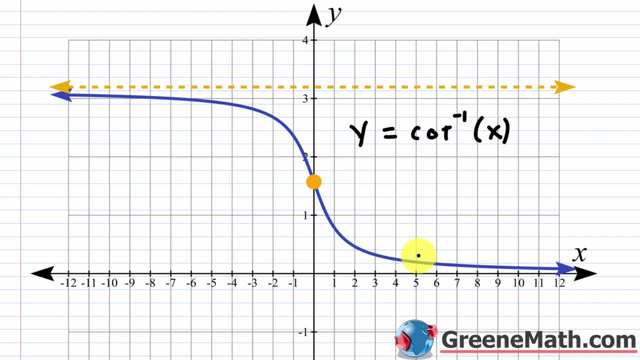 let's say from zero to pi, where zero and pi are not included, And basically, if you restrict that domain there you're going to get a one to one function And if you reflect that across the line y equals x, you're going to get this graph here. 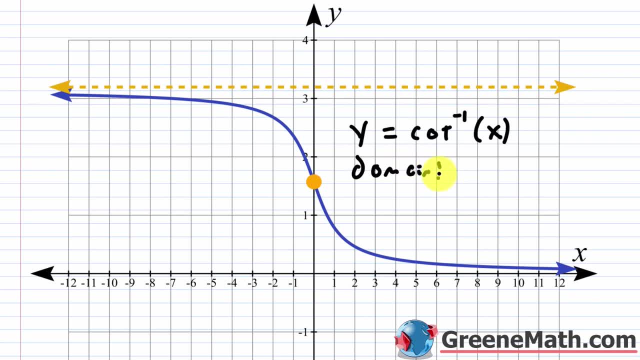 So in this case the domain is now going to come from the range of that guy. So you're going to have all real numbers, So from negative infinity to positive infinity, And then the range again is coming from the domain of that guy. 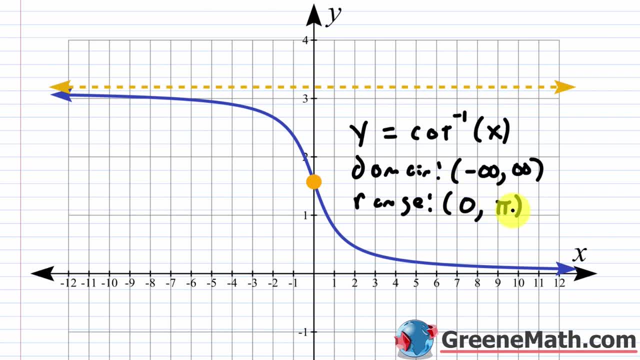 So from zero to pi, where zero and pi are not included. So the way you can evaluate this is to say it's x is equal to the cotangent of y, where y is greater than zero and less than pi. So again, zero and pi are not included. 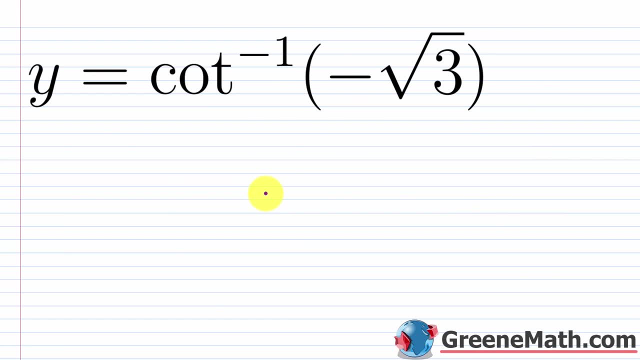 OK, let's look at a quick little problem And I'm going to show you an issue that's going to come up if your argument is negative for the inverse cotangent function. So we have: y equals the inverse cotangent of negative square root of three. 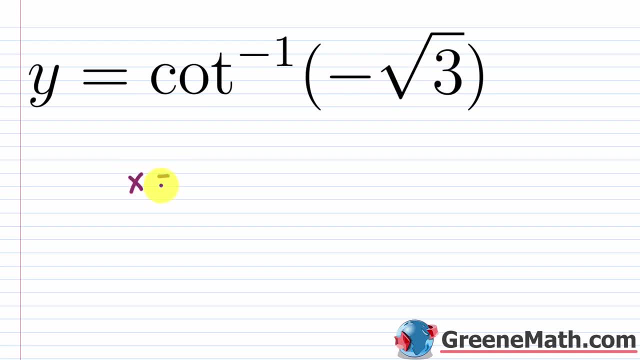 So, first off, I know that basically I can say that this is: x is equal to the cotangent of y, where y is greater than zero and less than pi. Well, the x here is the negative of the square root of three. So basically I'm asking for what angle between zero and pi is going. 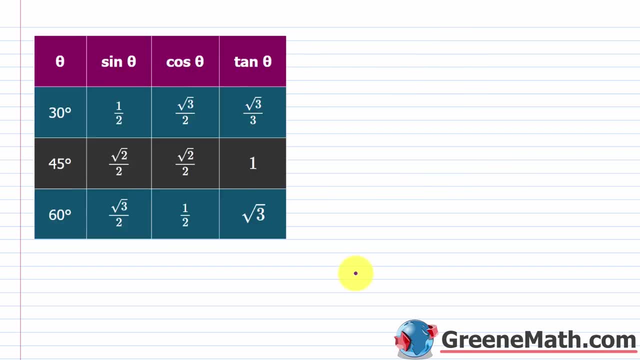 to have a cotangent value that's negative square root of three. Again, if you come back to this little table, some people have this for cotangent already, but I'm just going to use this one. If you look at this value right here for 30 degrees or pi over six radians, 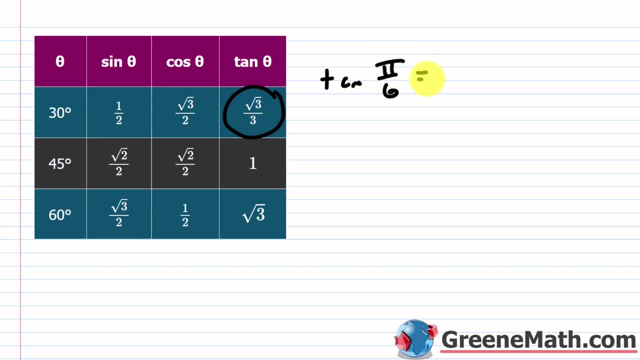 well, the tangent. so the tangent of pi over six is going to be the square root of three over three. So that tells me the cotangent of pi over six is going to be- again, take the reciprocal of this- so three over the square root of three. 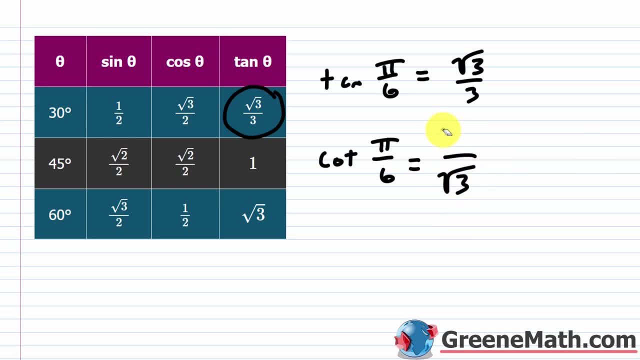 Now you could do this in different ways. You could rationalize the denominator, or a quicker way would be to say that three is the square root of three times the square root of three. So you could do it that way if you want. So this would cancel and you get the square root of three. 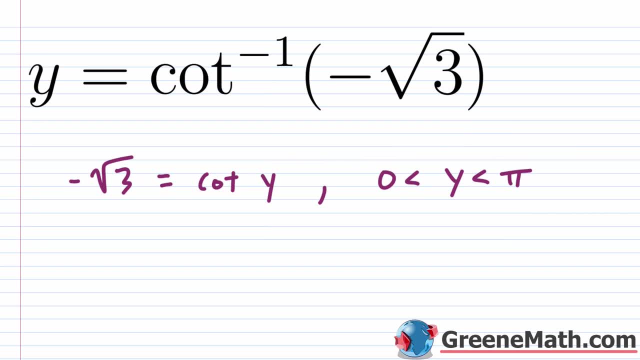 So pi over six would be my reference angle in quadrant two. So in quadrant two, what angle has a reference angle of pi over six? Well, it's going to be five pi over six. So this right here would just be equal to five pi over six. 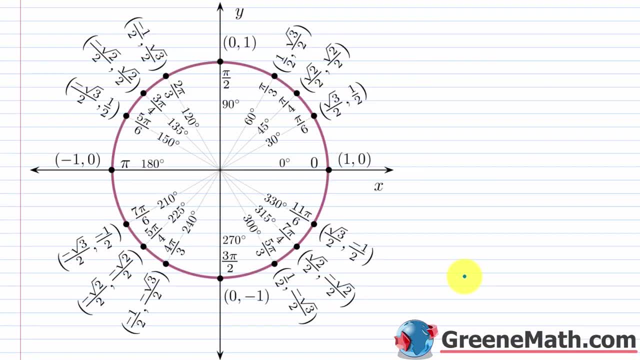 Again, it's got to be within this interval for you to give that answer. Another way you could have done this is by using the inverse tangent function. So let's say you started with the inverse cotangent of your negative square root, And let me make that a little bit easier. 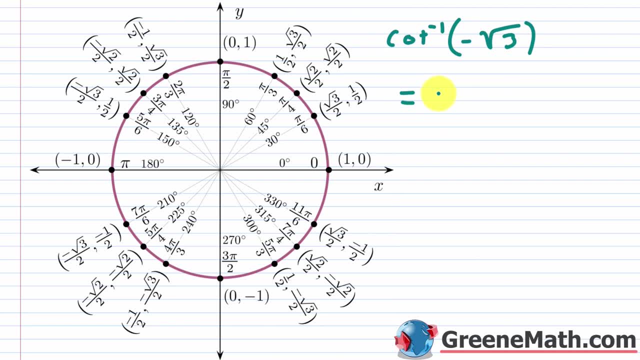 A little bit better. Of three, Can you say this is equal to the inverse tangent, So the inverse tangent of the reciprocal of this, So the negative of one over the square root of three. If you rationalize the denominator, that is the square root of three over three. 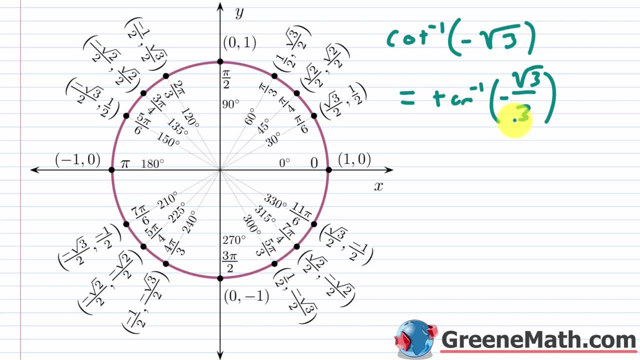 Well, the answer to that question is no. You need to issue a little bit of a correction, because this right here- So this right here- is going to give you something in quadrant four, rotating clockwise. So this guy right here, I'm going to give you this guy right here. 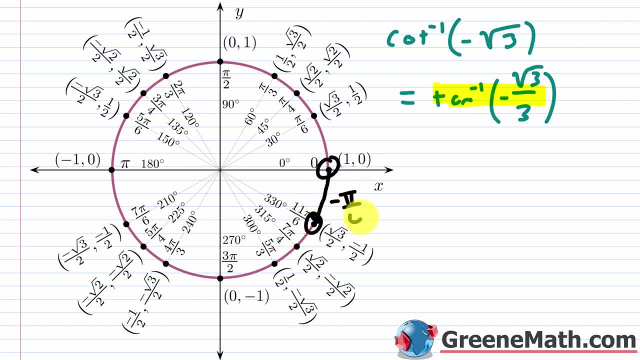 So this would be negative pi over six. So a pi over six. reference angle in quadrant four And you've got to rotate clockwise. But the answer is actually going to be right here at five. pi over six, because with the inverse cotangent function I'm working from zero to pi. 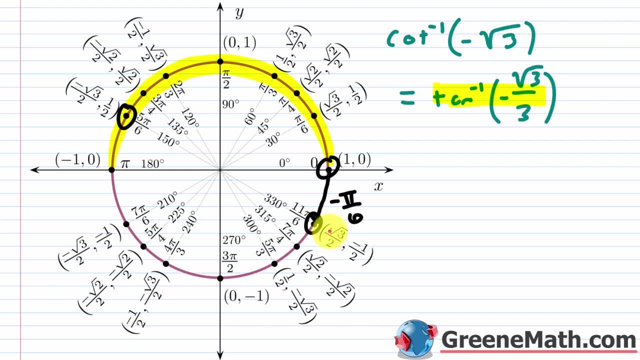 So I'm working right here. So what you would want to do is make yourself a little correction and add pi. So I'm going to add pi so I can swing around Right there, And that's going to give me the correct answer. 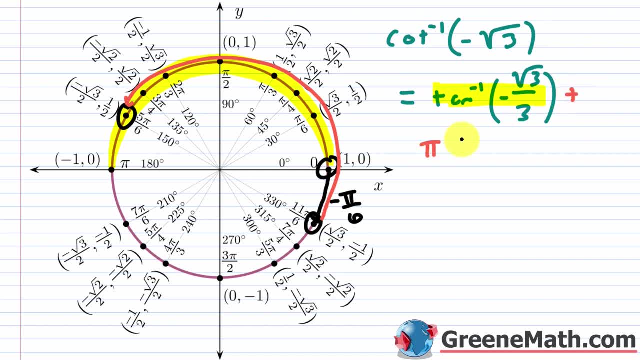 So I'm going to add pi to issue a correction here, And so this would be negative pi over six plus pi. Let's write that as six, pi over six, And so that would be equal to the five pi over six. That is the correct answer. 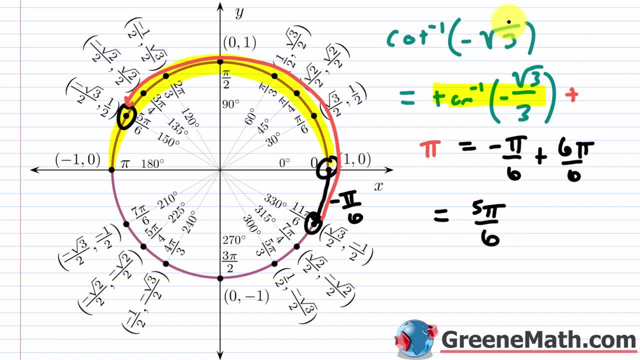 So if you're using your calculator, you need to be aware of this. If your argument is positive, you're going to be in quadrant one, So you're OK there. You don't have to issue a correction because the inverse tangent of something. 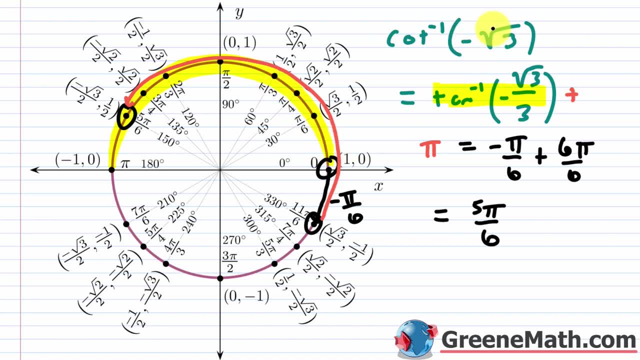 that's positive is going to give you something in quadrant one as well. But if this guy is negative, you're getting something in quadrant four for the inverse tangent function and you're getting something in quadrant two for the inverse cotangent function. So you have to be very, very careful and issue a correction there. 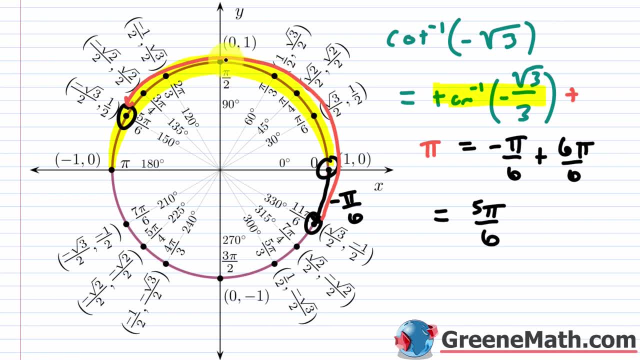 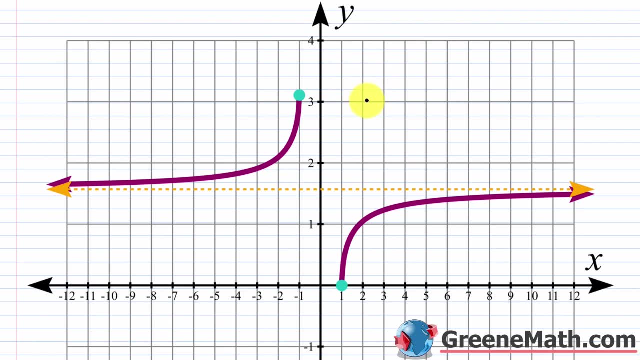 Now, if you do the inverse cotangent of zero, you're just going to end up getting pi over two as an answer. So that's one you just need to memorize, All right. So the next graph is going to be for the inverse secant function. 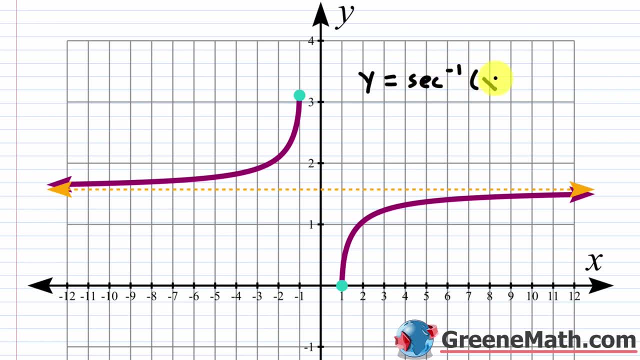 So y equals your inverse secant of x. So if you look at the domain, so the domain So this one. let's just do it in interval notation. So from negative infinity to negative one. So let's go from negative infinity up to and including negative one. 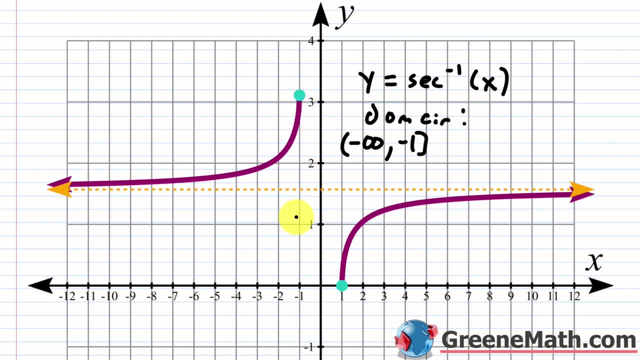 So again, this is included here. You have a point there. This would be negative one comma pi And then basically the union with positive one is included and out to positive infinity. So basically the values between and not including negative one and positive one. 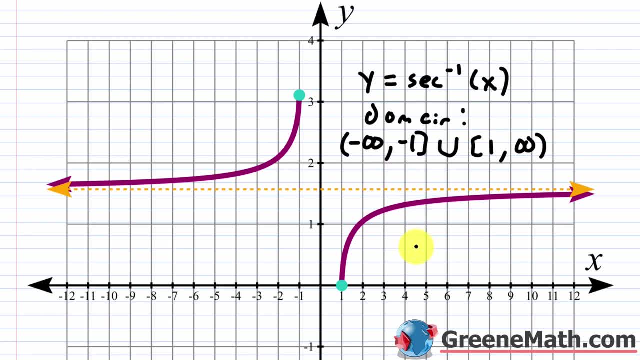 Those are excluded from The domain. So then for the range, let me write that down here. So for the range, you can see that this guy is going to be from zero to pi, where basically this pi over two. Let me write this in So this is not confusing. 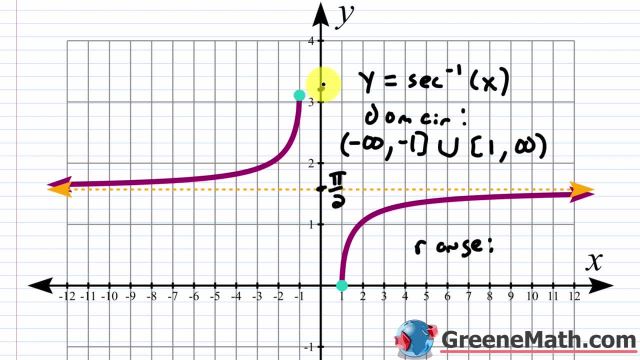 So this is pi over two here. That's not going to be included. Let me write up here that this is going to be pi, So the range you're going to have. We move this up a little bit So it fits basically from zero and including zero going up to and excluding pi over two. 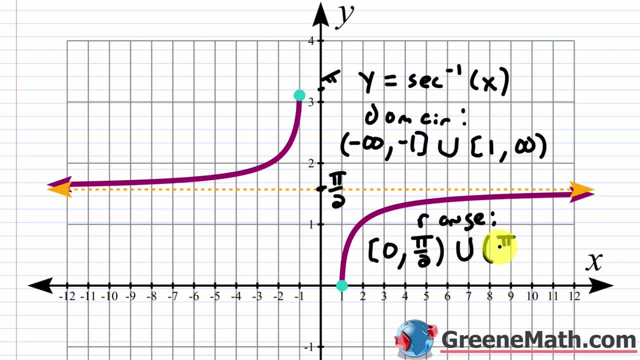 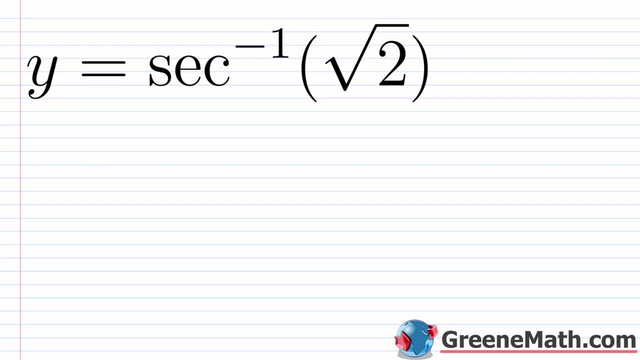 And then the union with You're going to have again pi over two is excluded, going up to and including pi. OK, let's take a look at a little sample problem. We're going to convert this over and solve it very quickly. 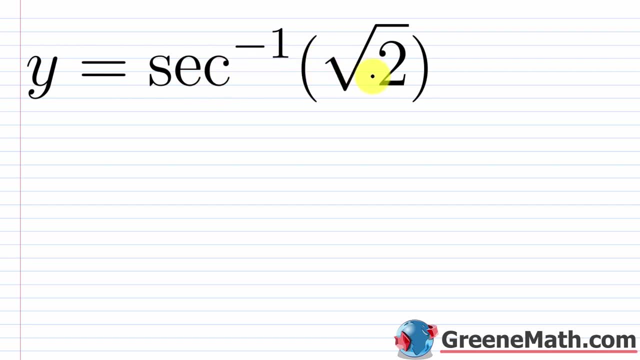 So here we have: y equals the inverse secant of square root of two. So essentially, what I'm going to do is actually say that this is equal to the inverse cosine of. I'm just going to take the reciprocal of this, So one over the square root of two. 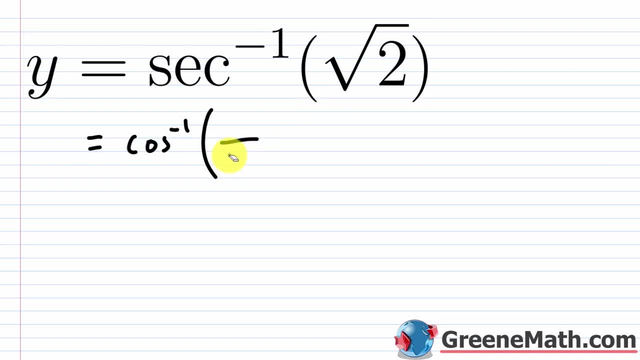 So if you rationalize the denominator there, this becomes The square root of two over two, And so this, we know, is going to be pi over four. So for these problems you don't have to issue a correction. Basically you're just going to key it in like this: 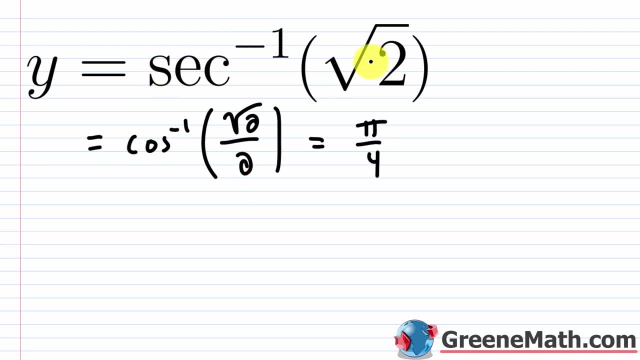 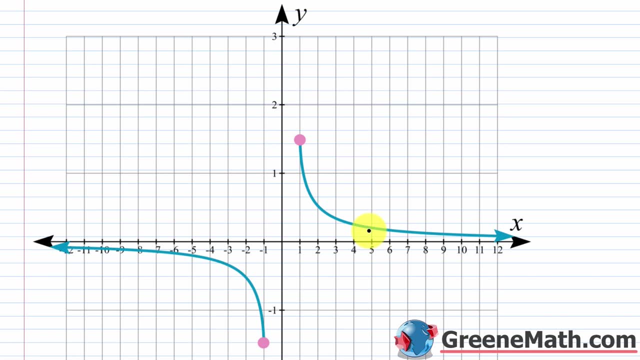 So if you have the inverse secant of something, you basically are going to take the reciprocal of that value and have the inverse cosine of that, And that's how you're going to get your answer. All right, let's take a look at the inverse cosecant function. 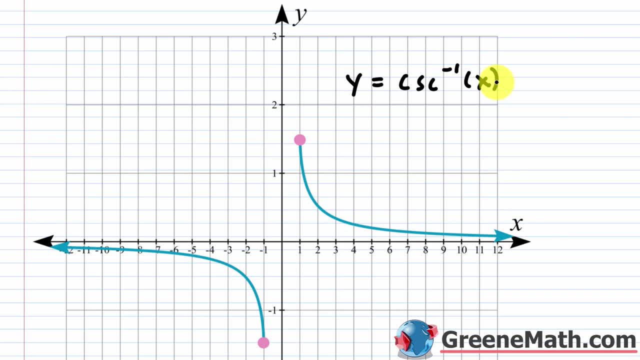 So again with the inverse cotangent function, the inverse secant function and the inverse cosecant function, it might look different in your book or your online resource, so just telling you that in advance. So this guy right here for the domain, pretty easy to see. 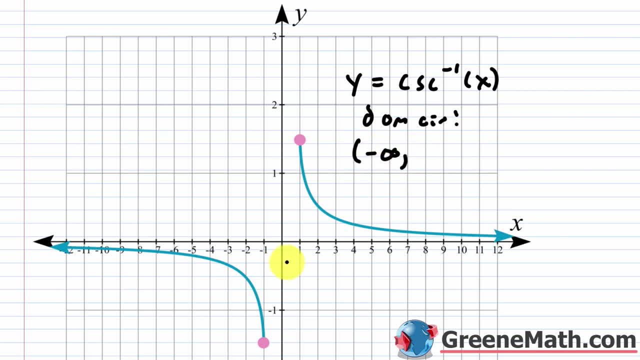 Basically it's going to be from negative infinity up to and including negative one. So this right here, this is a point that's included. So this would be negative one comma, negative pi over two And then basically the union with this point right here. 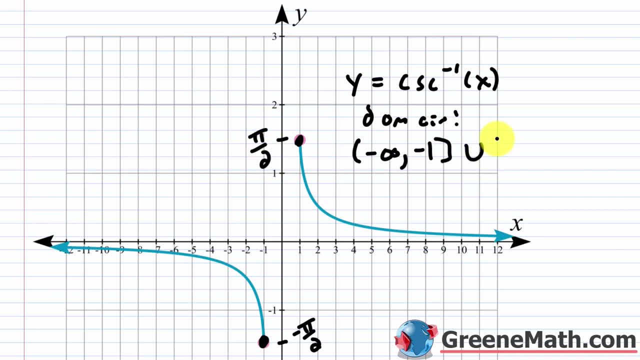 This is positive one comma pi over two. So basically, you're going to take From positive one out to positive infinity. so that's your domain. And then in terms of your range. so in terms of your range, well, that's going to be from negative pi over two to pi over two. 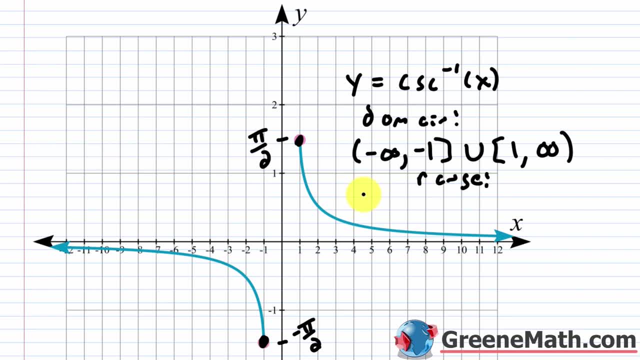 where you're going to exclude zero. So basically let's say we have from negative pi over two and then we're going to go up to and exclude zero, And then the union with: again we're excluding zero and we're going up to pi over two. 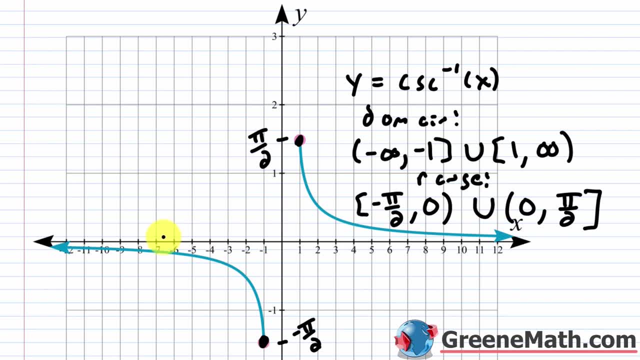 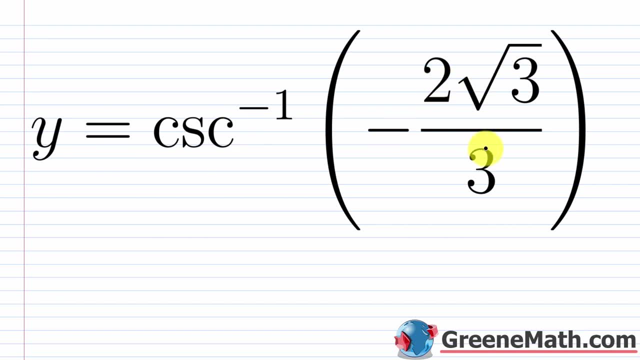 So pi over two and negative pi over two are included, but zero here That's going to be excluded. OK, let's look at a problem. So here we have: y equals the inverse cosecant of a negative two times square root of three over three. 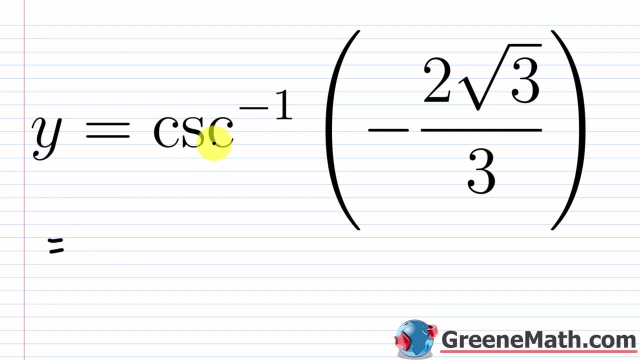 Again, all you have to do for this problem is say this is equal to: I'm going to use my inverse sine function, so my inverse sine function, And I'm just going to take the reciprocal of the argument here. So it's going to be the negative of three over two times the square root of three. 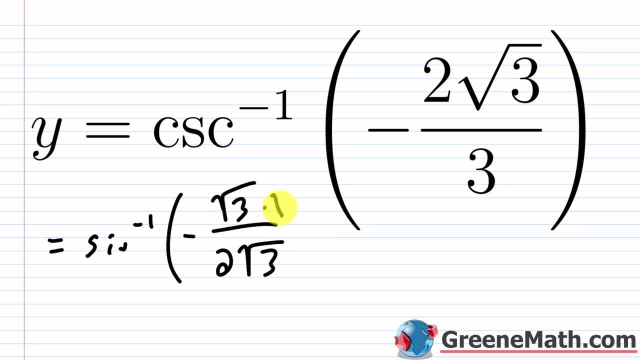 So let me go ahead and write this as the square root of three times the square root of three, And I'm going to cancel this with this, And so this becomes the negative of square root of three over two, So the negative of the square root of three over two. 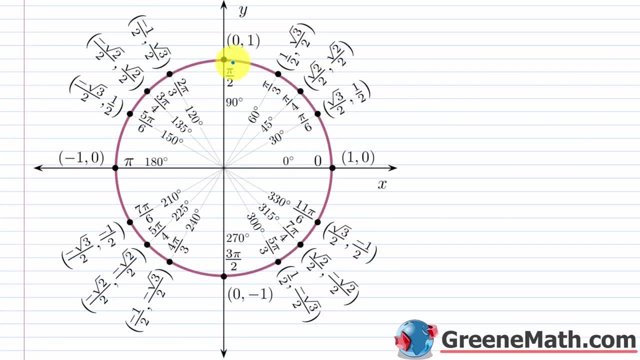 And this one might benefit a little bit from the unit circle. So again, with the inverse sine function, you're working in quadrants one and four. If you're in quadrant four you've got to rotate clockwise. So where is my sine value? negative square to three over two. 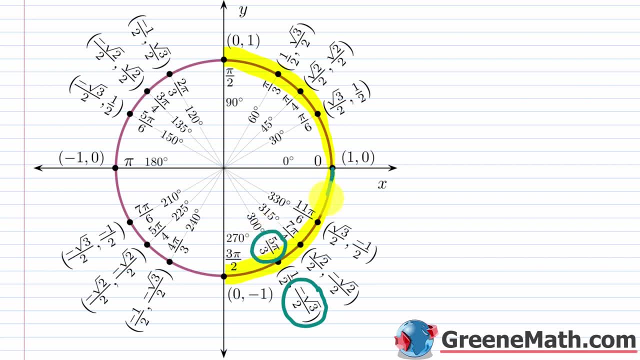 It's going to be right there at five pi over three. But again you've got to rotate clockwise. So the reference angle there is pi over three. So you'd say this is negative pi over three. So that's what you want for your answer. 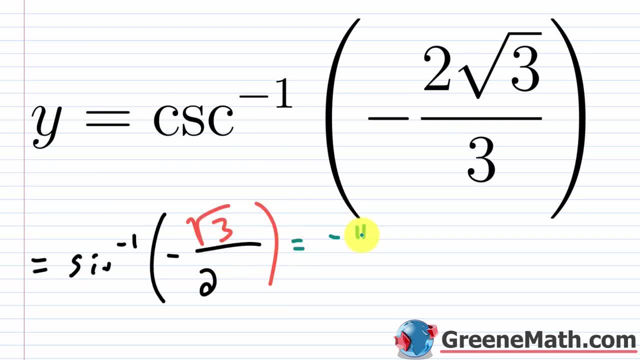 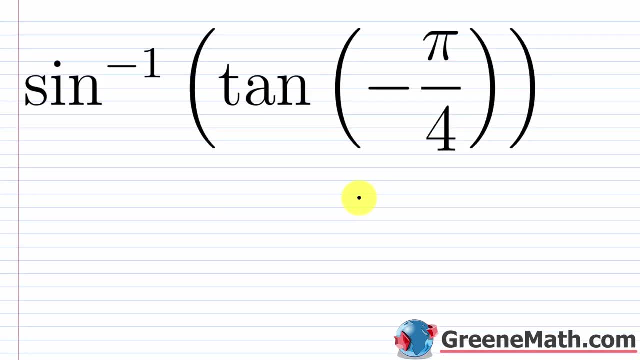 Let me just move this down here. This would be equal to negative pi over three. So these types of problems are really easy. if you already understand the inverse sine function, All right. Now let's move on and look at some typical examples for this section. 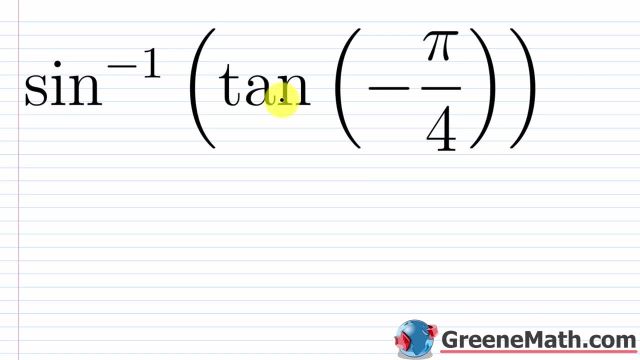 So what if you see something like the inverse sine of the tangent of negative pi over four? Well, the idea for this type of problem is to evaluate this part first. So what's inside, or what's going to be, the argument for the inverse sine function? 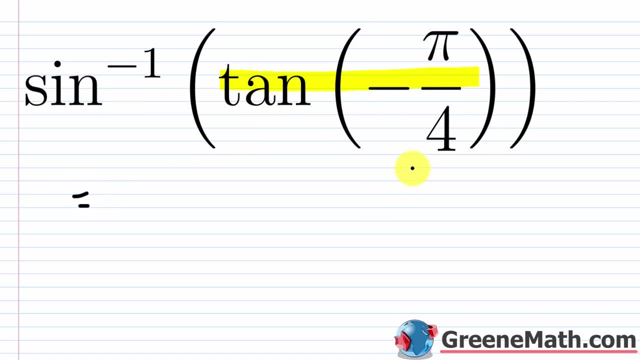 And so you would say: what is the tangent of negative pi over four? A lot of you know that's negative one, But again, just in case you don't, you're going to look at your unit circle and you're going to say: well, 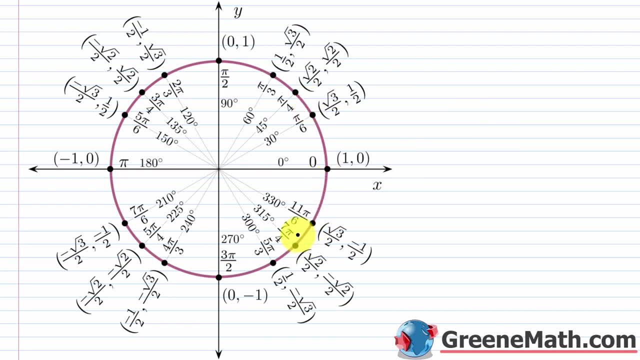 where is negative pi over four? Well, again, I'm looking in quadrant four and I want a pi over four reference angle. So that's going to be right here at seven pi over four. But what I'm doing is I'm rotating clockwise. 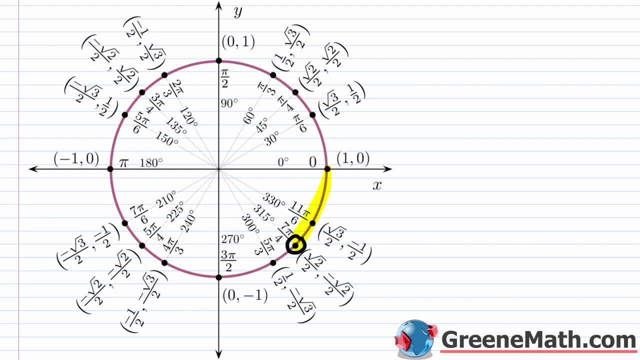 So I want this guy right here again rotating clockwise. Let me do this in a different color here, So this shows up really well. So this right here is the angle that I'm looking for: Negative pi over four. Now, of course, this is coterminal with seven pi over four. 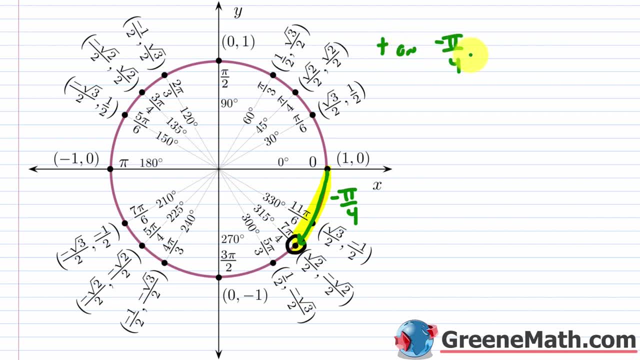 So if I want the tangent of negative pi over four, I can just say that equal to the tangent of this seven pi over four, And I could just grab that from the unit circle again. here You want the sine value, which is negative square root of two over two divided by the cosine value. 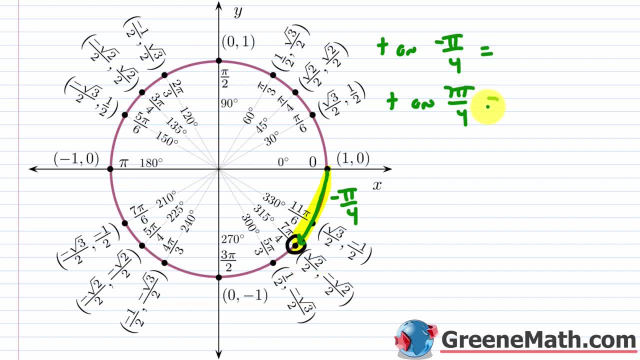 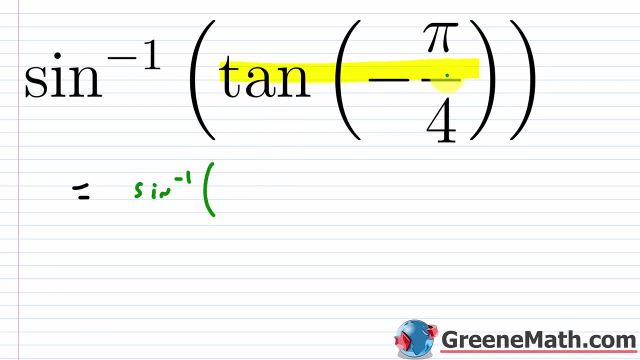 which is square root of two over two. So I'm dividing opposites, So I'm going to I'm going to get negative one as a result. So, coming back up, this would be the inverse sine of this. right here is negative one. 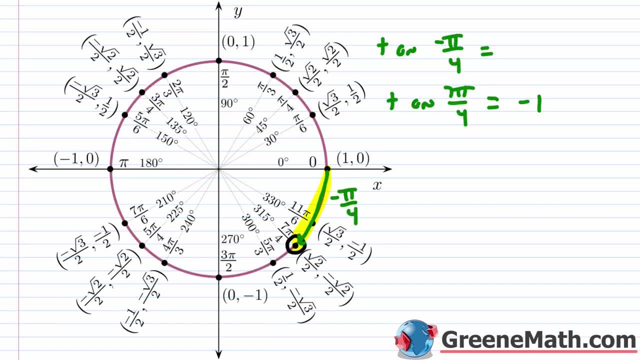 And again, a lot of you already know this is going to be negative pi over two. But again, because we just started with this section, let me get rid of this. You're thinking about where your sine value is negative one, So that's going to be right here. 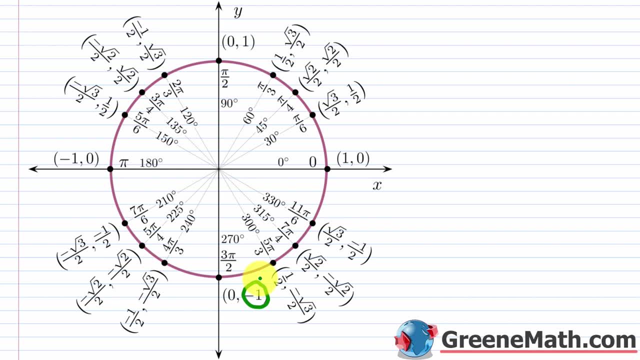 But again, that's not in the interval of the inverse sine function, So I can't give this three pi over two as a result. So what I want to do is think about rotating clockwise, So clockwise like this, And basically that's going to give me an angle that is negative. pi over two. 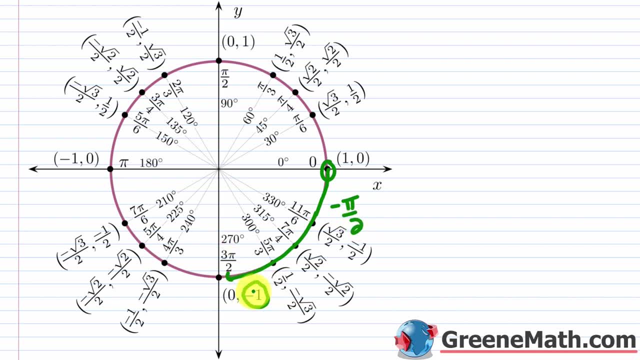 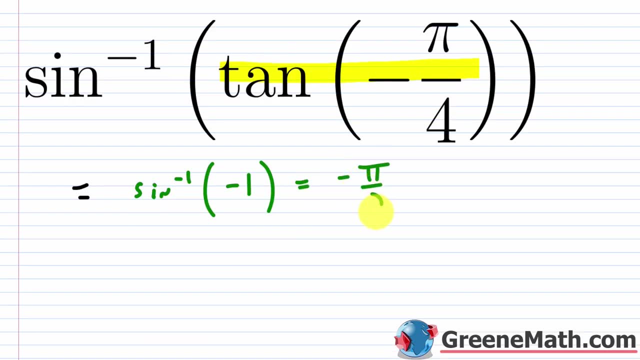 And of course that's coterminal with three pi over two. So the sine value is going to be the same, It's going to be negative one. So, coming back up, I want to give an answer here. That's going to be negative pi over two. 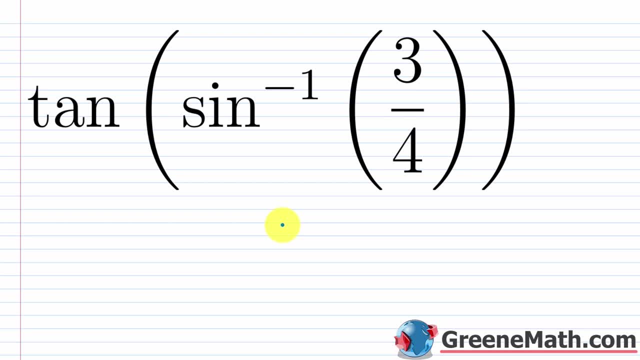 All right, Let's look at another common type of problem for this section. So you might see something like the tangent of the inverse sine of three fourths. So what can you do for this type of problem? Well, of course, you could pull out your calculator. 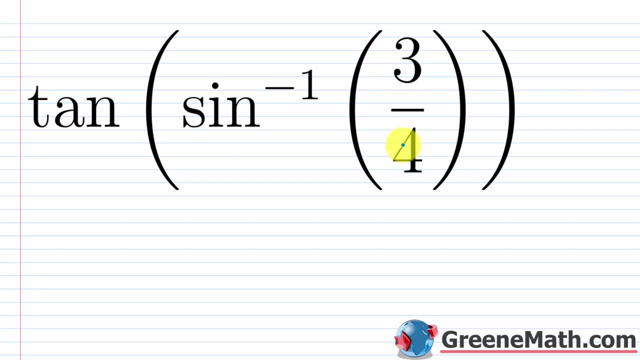 And you can key in the tangent of the inverse sine of three fourths And it will give you an approximation, But in most cases you're asked to find the exact value. So for that, what I recommend is to make a little substitution for this part right here. 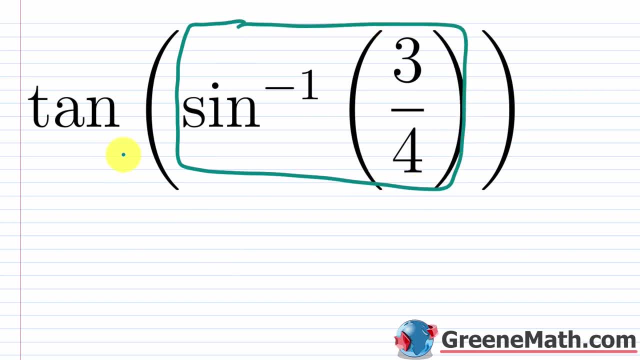 So the inside, right here, which is the argument for the tangent function, you're going to let something like, let's say, theta be equal to this guy right here. So the inverse sine, So the inverse sine of three, fourths And so 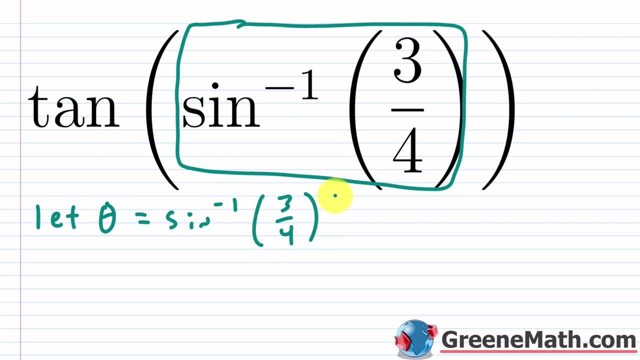 Since theta is equal to this, I can say that now I'm trying to figure out what is the tangent of theta. So I'm just going to say, for right now, this equals what? So let me slide down and let's think about: do we have enough information to figure out what the tangent of theta is? 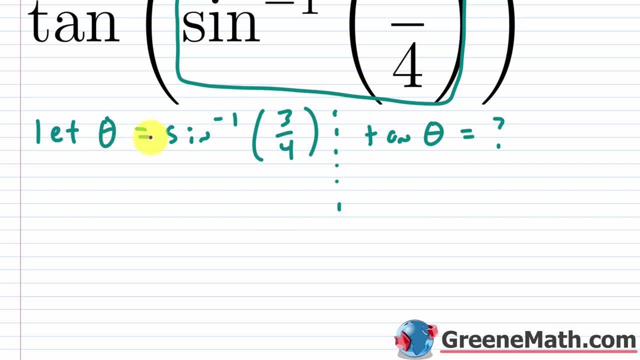 Well, of course we do. First off, we know that if theta is equal to the inverse sine of three fourths, then we can say, So I'm going to put. then we can say that the sine of this angle, theta is equal to my sine value is three fourths. 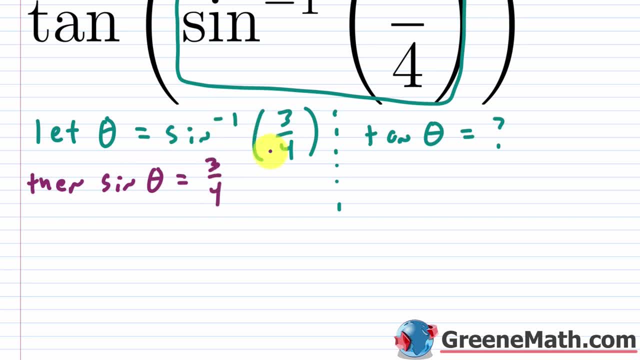 Again, if the sine of theta is three fourths, well then the inverse sine of three fourths is going to get me back to theta. Now we also know that a sine is positive. I'm going to be in quadrants one or two. 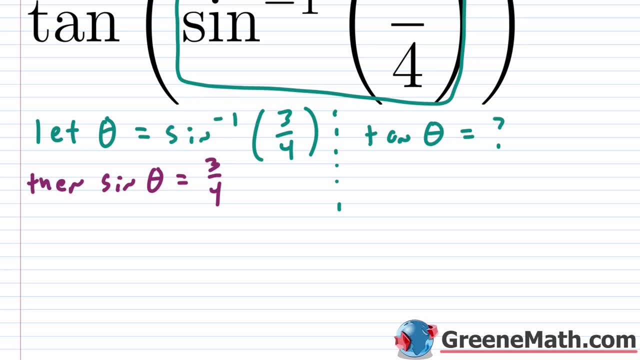 But specifically here, because I'm working with this inverse sine function and the argument is positive here. I know I'm going to be in quadrant one. This is always going to be true, unless you have the inverse sine of positive one, which is pi over two. 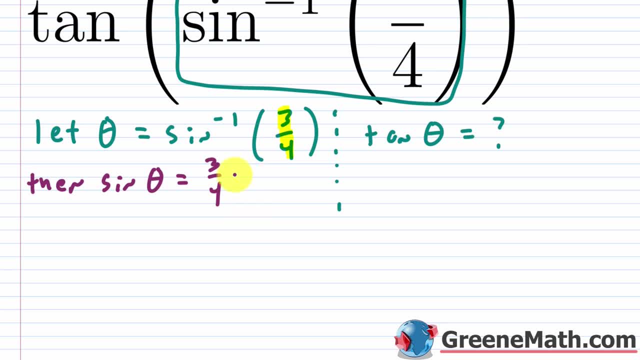 That's a quadrantal angle, but that's the only exception. So for this particular case, we know that theta is in quadrant one and I went over my border a little bit. So let me put the border like this. And so now I can go back to what I talked about earlier on in the course, when we 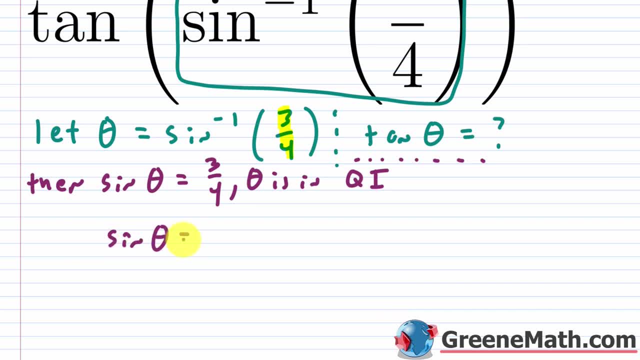 said that, OK, if the sine of theta is equal to three fourths, well, that three is going to be your opposite or your Y, and that four is going to be your hypotenuse or your R. So if I want to figure out the tangent of theta, 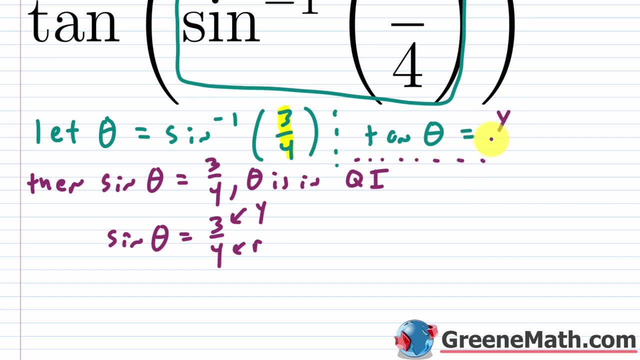 remember this is going to be your Y or your opposite, over your X, which is your adjacent. So I already know that Y is three. So I can just plug that in right now and say this is three And I just need to figure out what is X. 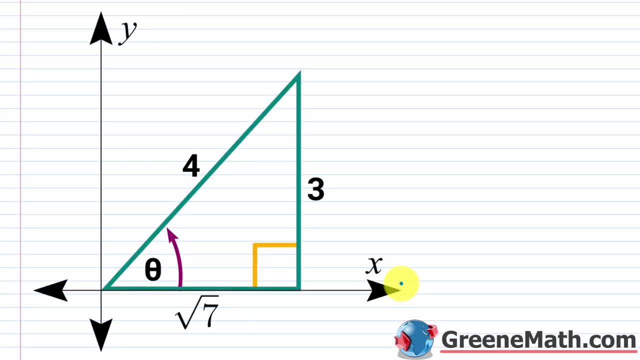 So you're going to use your Pythagorean theorem? You don't have to do this, but I went ahead and made a little sketch. So remember, for the Pythagorean theorem you have X squared plus Y squared is equal to R squared. 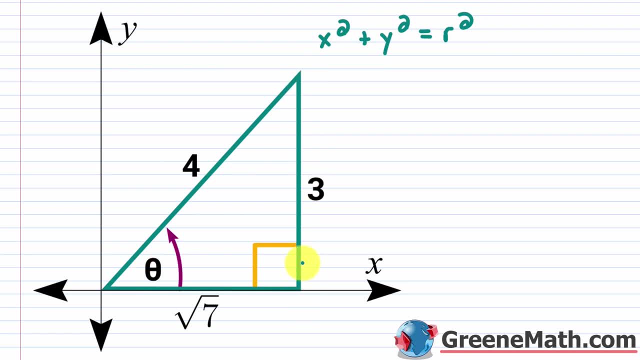 So in this case, we know that the Y, or the opposite side, is three, So I'm just going to plug that in there. We know that the R, or the hypotenuse, is four, So I'm going to plug that in there. 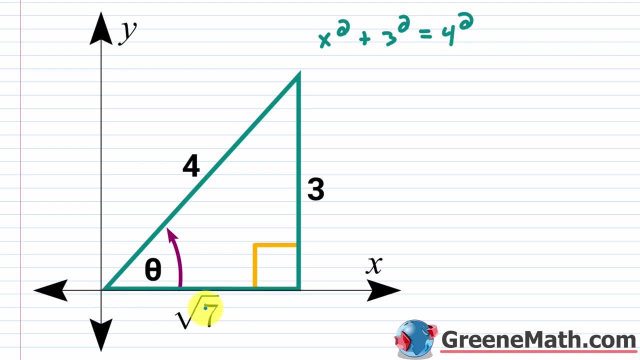 We're going to find that the X or the adjacent side is going to be square to seven. Right now I don't know that. I'm going to solve for that. So here I would have: X squared plus three, squared is nine, And this equals four squared, That's 16.. 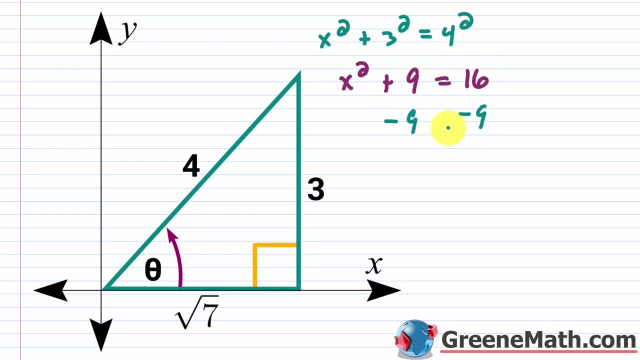 So what I'm going to do is subtract nine away from each side of the equation, And so this right here is going to cancel. You'll have X. squared is equal to 16 minus nine is seven. Now, by the square root property, you would say that X is 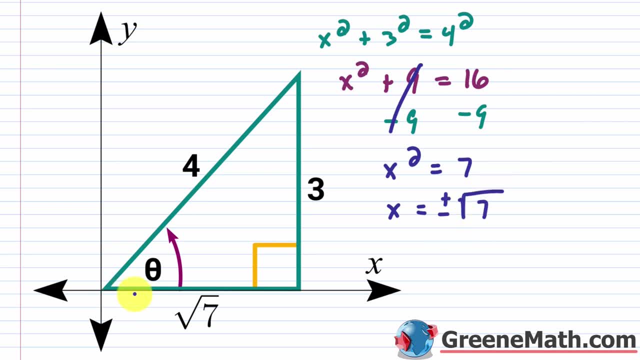 equal to plus or minus the square root of seven. Now in quadrant one where X values are positive, So I don't need the plus or minus here- X is going to be the principal square root of seven. So now I know that the adjacent side here 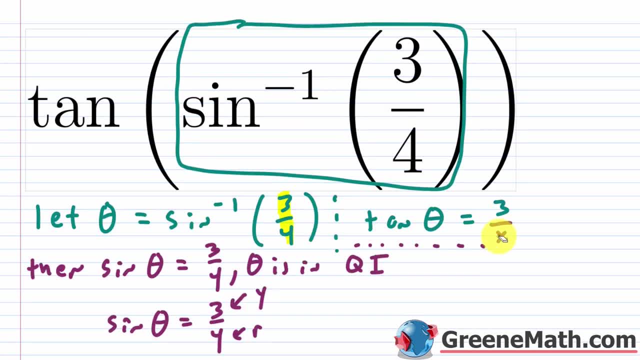 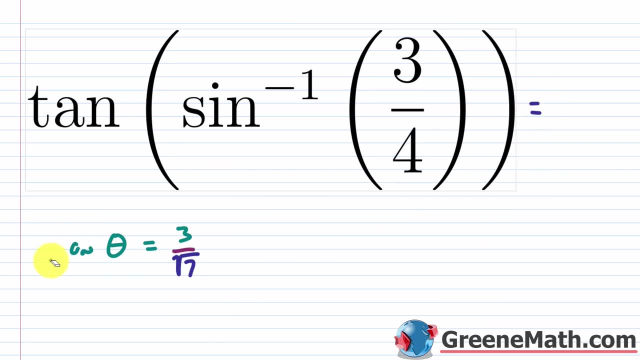 or the unknown X is going to be square to seven and just coming back up, I'm going to put that this right here is the square root of seven And let me move this over here. I can just answer that this right here is three over the square root of seven. 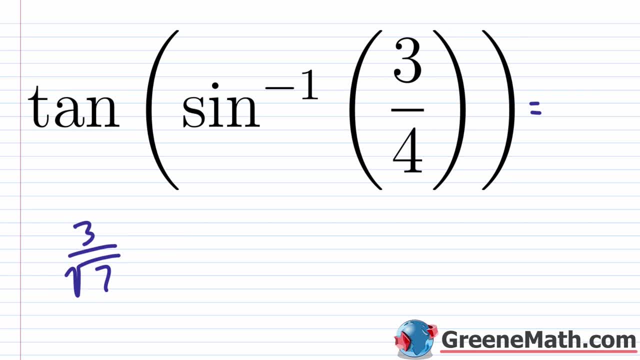 So three over the square root of seven. And of course you would want to take the denominator So times the square root of seven over the square root of seven. So my final answer here for the tangent of the inverse sine of three fourths is going to be three times the square root. 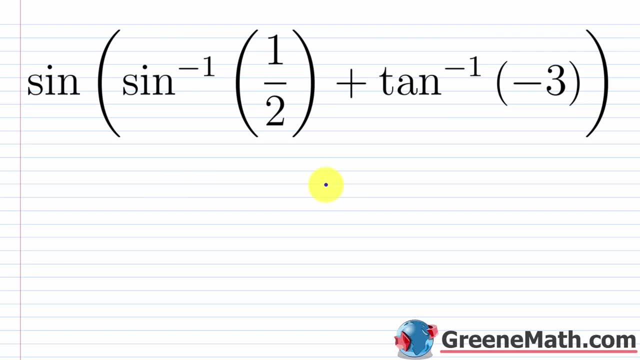 of seven over seven. All right. Now let's look at another type of problem. So this one is just a little bit more tedious than the previous problem. So we have the sine of the inverse sine of one half plus the inverse tangent of negative three. 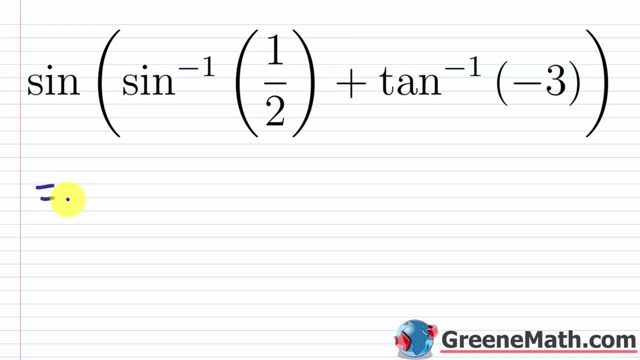 So for sure you're going to get a problem like this in your textbook And what you want to do is start off by asking: can I replace anything in my problem? So in other words, I know that the inverse sine of one half is pi over six. 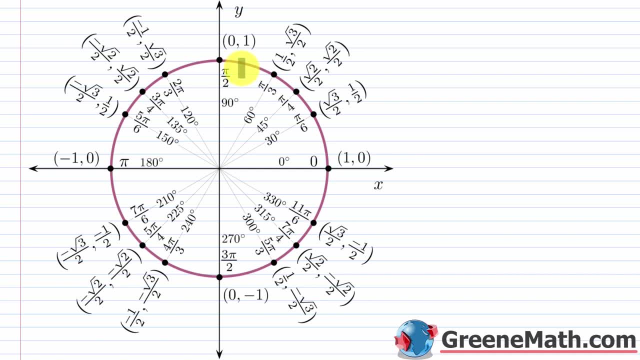 Let me just come down to the unit circle. again This is new for us. I know a lot of you already know that. But again I'm working from negative pi over two to pi over two And I am asking the question: what is the inverse sine? 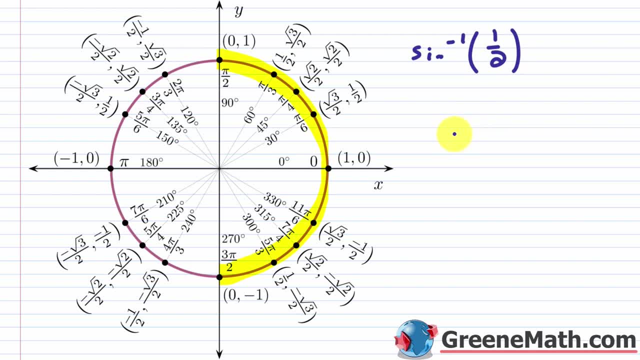 So what is the inverse sine of one half? So I'm looking for a sine value of one half. So that's going to occur right here, And so what I want for the associated angle is pi over six. So the sine of pi over six is pi over six. 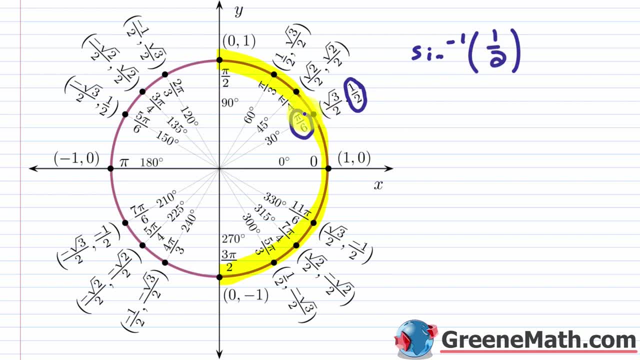 So the inverse sine of one half is going to be pi over six. Again, it's got to be in this interval from negative pi over two to pi over two. So this right here is going to be pi over six. So, coming back up here, I'm just going to replace this with pi over six. 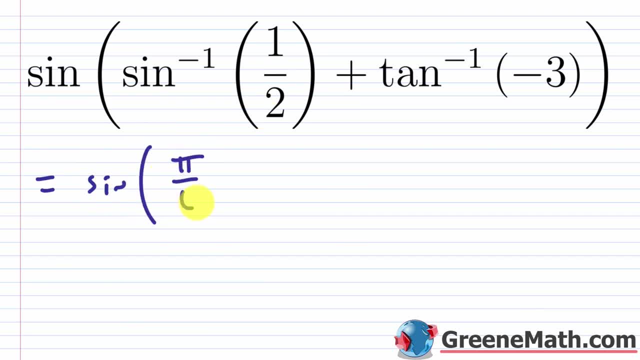 So this is the sine of your pi over six, plus Now this one. I'm going to make a substitution for it. Let me just write it in for right now. So the inverse tangent of negative three. OK, so, just like in the previous, 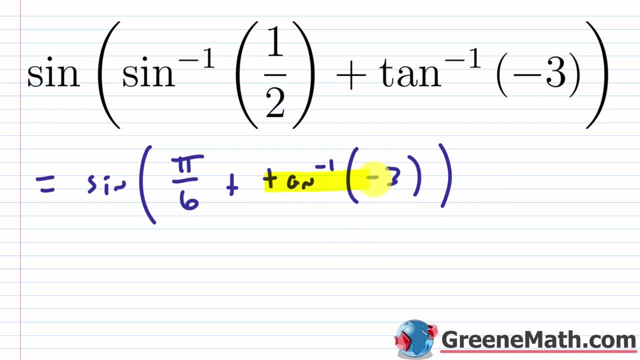 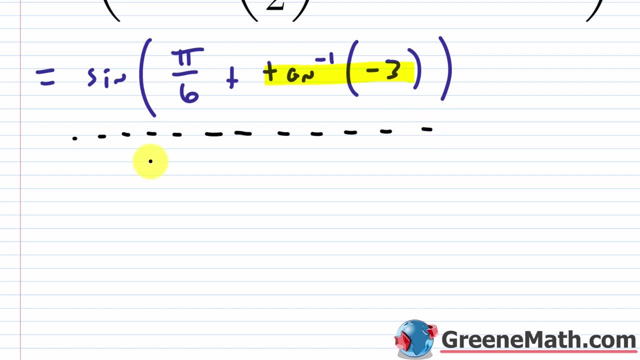 problem. we have something here where we're going to make a little substitution, So you have the inverse tangent of negative three. Let me slide down here real quick And I'm just going to put that. we are going to let something like beta be equal. 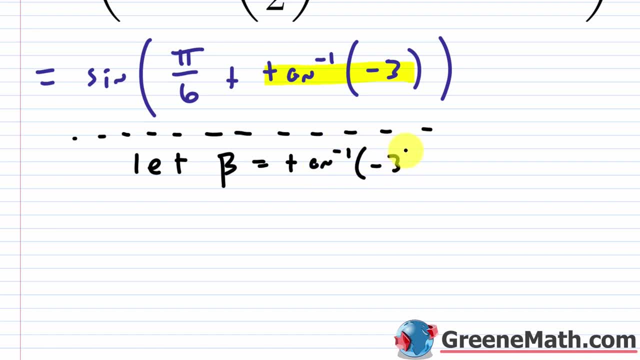 to the inverse tangent of negative three. So what I'm going to do is replace this right here with beta. So I'm going to say that now I'm looking for the sine of pi over six plus beta. Remember, when we think about this beta here. 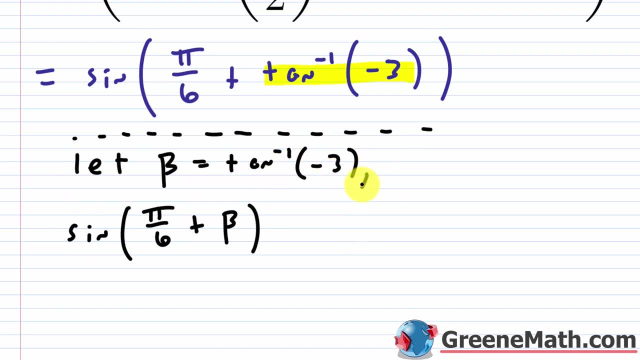 if we let beta be equal to the inverse tangent of negative three, that tells me that the tangent of beta is equal to negative three. Now where is beta? Remember, the inverse tangent function is going to give you something in quadrant four, rotating clockwise, if the argument is negative. 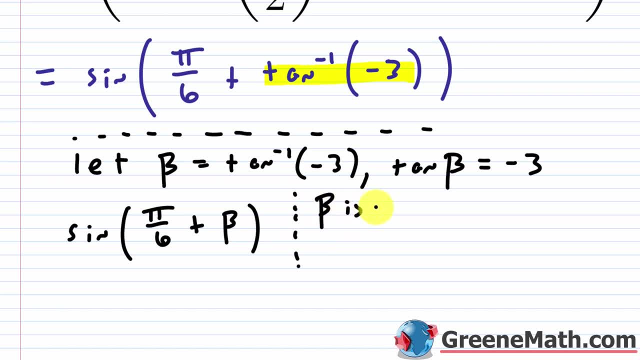 So that tells me- let me put a little border here- that beta is in quadrant four. OK, so we're going to use that in a little while. So the first thing is I'm going to grab this and copy it and I'm going to go to another page. 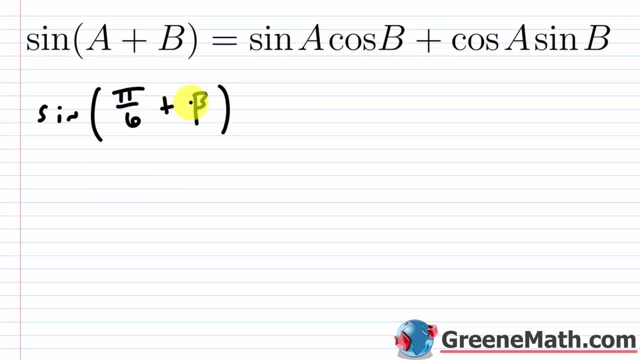 And let me paste this in here: When you have the sine of A plus B- in this case it's pi over six plus beta- But the sine of A plus B is equal to the sine of A times the cosine of B plus the cosine of A times the sine of B. 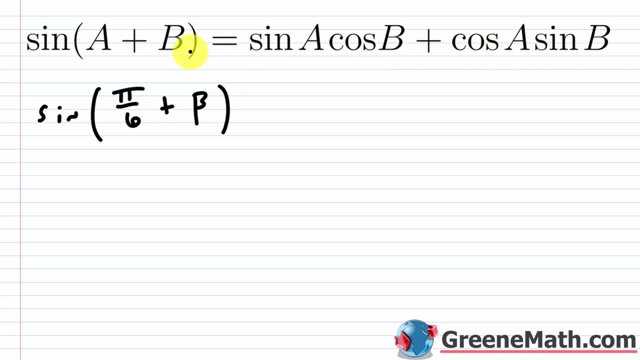 This is your sum identity for sine that we talked about earlier in the course. So we're going to say that this sine of you have, this pi over six plus beta, This is equal to the sine of the first guy, which is pi over six and then times the. 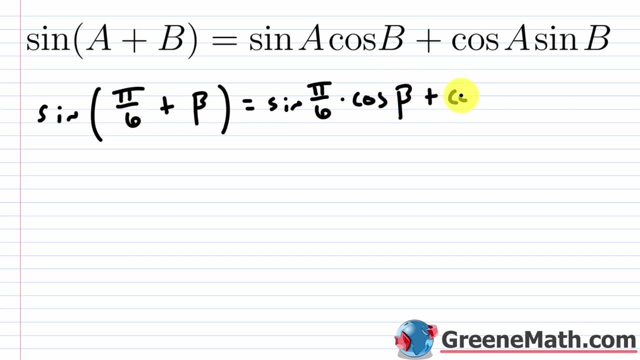 sine of the second guy, which is beta, and then plus the cosine of the first guy, which is pi over six, and then times the sine of the last guy, which is beta. So the sine of beta. So this equals what In terms of the sine of pi over six? we know that's a half. 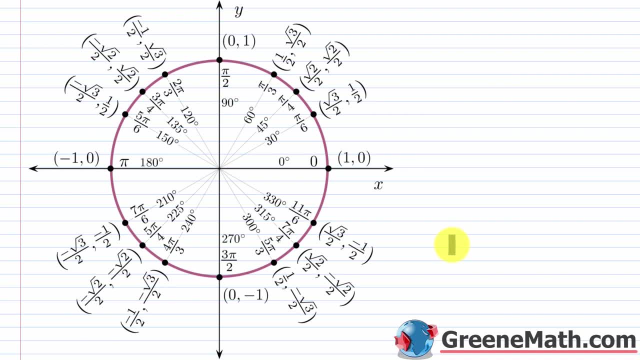 And the cosine of pi over six. that's square root of three over two. Most of you don't need this at this point, But again, if you don't have a unit circle, here's pi over six. So the sine value is one half and the cosine value is square root of three over two. 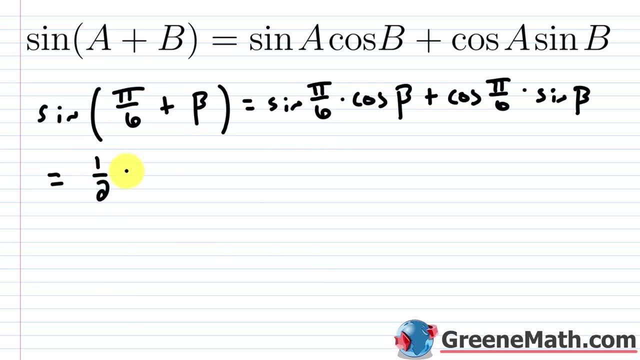 So let me come back up here. So the sine of pi over six is one half and then times your cosine of beta, And then, plus the cosine of pi over six, is the square root of three over two, and then times your sine of beta. 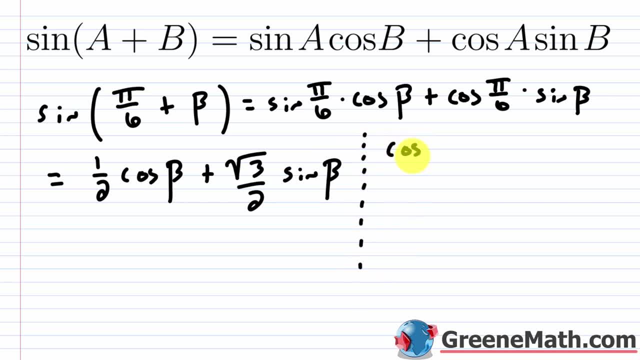 So what I need to do is I need to figure out what is the cosine of beta. So the cosine of beta is again, that's your adjacent over your hypotenuse, or we say the X over the R. And then what is the sine of beta? 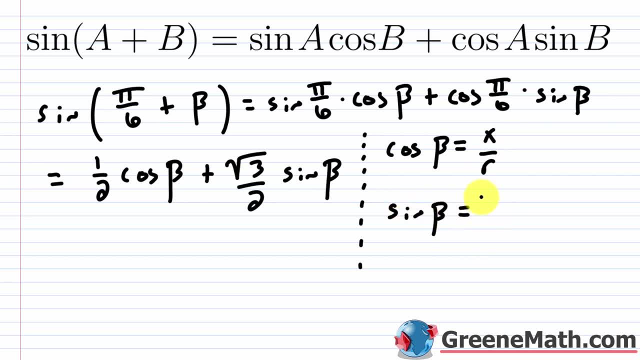 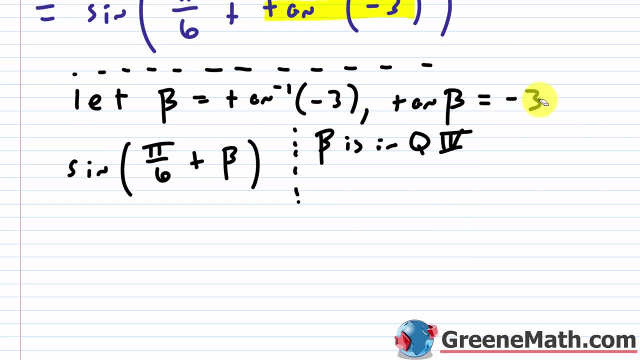 So the sine of beta is equal to your opposite over your hypotenuse, or your Y over your R. Well, let's go back up and let's remember that we know that the tangent of beta is equal to negative three. You can go ahead and say that this is negative. 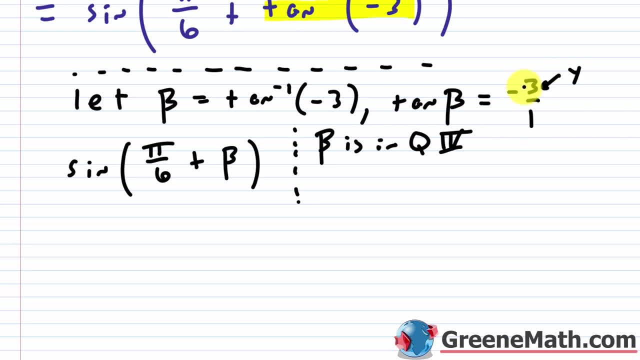 three over one. So this right here is the Y value. It's going to be negative three because again we're in quadrant four. So the Y values are going to be negative and the X values are going to be positive, And this right here will be your X value. 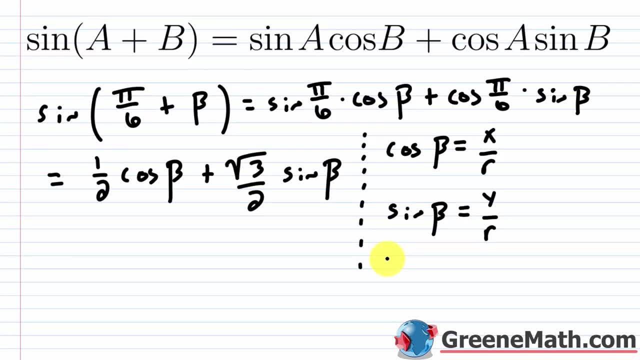 So that's positive one. So let's come down here. I'm just going to write in that the tangent of beta is equal to negative three over one. Again, this is your Y and this is your X. So we can come through here and say that X is one. 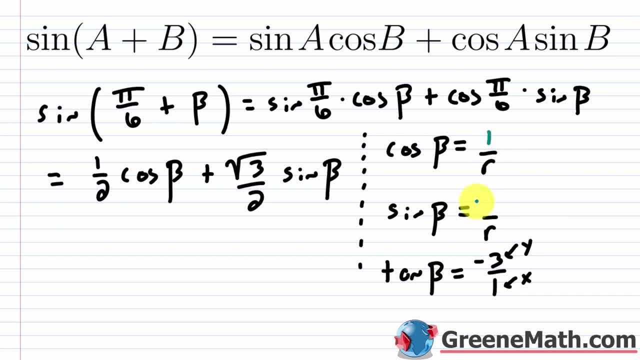 So I know this is a one, and then Y is negative three. So I know this is negative three. Now how do we get R Again? go back to the X squared plus Y squared equals R squared And again you can make a sketch. 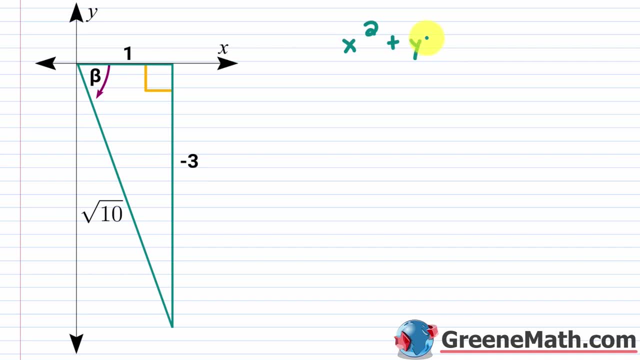 It's not necessary, but you can do it. So let's put X squared plus Y squared equals R squared. We're going to find out that R, or this hypotenuse here, is square to ten. But to get that X or your tangent is going to be positive one. 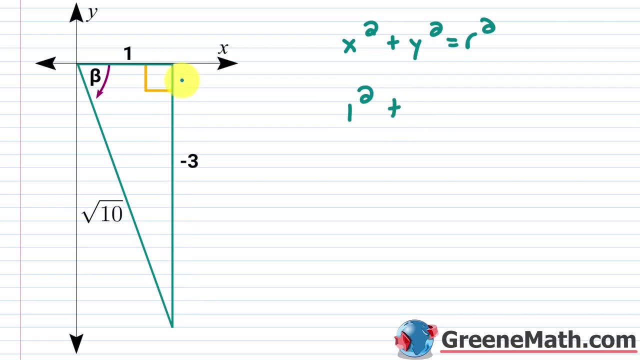 So this is one squared plus your Y, or your opposite, is going to be negative three. Remember you're in quadrant four, So the Y values are negative. So this is negative three. Make sure to wrap that. and this is going to be squared. 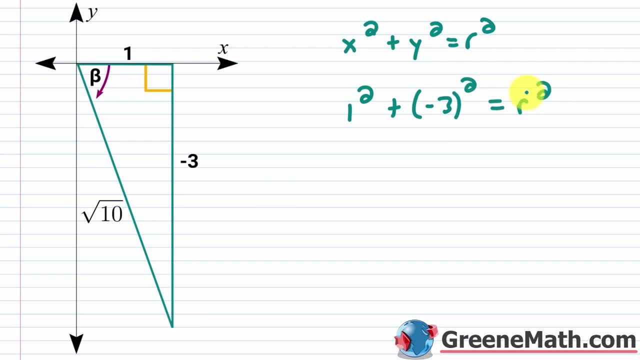 And this equals your R being squared. So that's going to be, for your hypotenuse, that guy being squared. OK, so this is pretty straightforward: One squared is one, and then plus negative three- Again this is wrapped being squared. 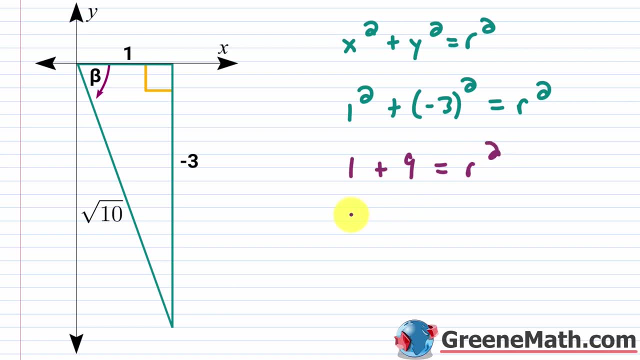 That's positive nine And this equals R squared. So you get R squared is equal to ten. Again, by the square root property, you get R is equal to plus or minus the square root of ten. Now your R is always positive. 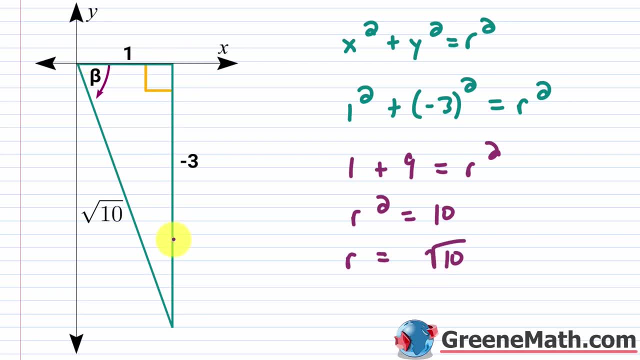 So this is just the principal square root of ten. So your X is one, your Y is negative three and then your R is going to be square root of ten. So, coming back up, if I know that R is square root of ten, 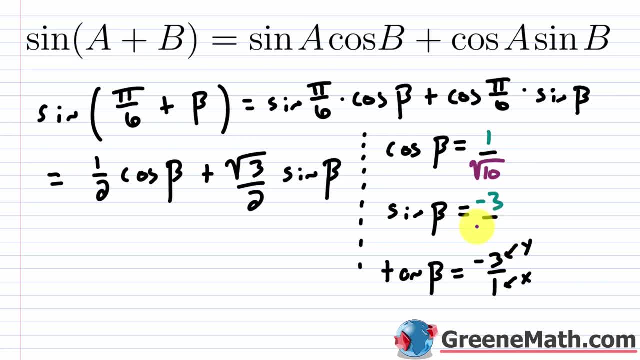 I'm just going to replace that here. So this is square root of ten, And then this right here is square root of ten. OK, I'm going to get rid of this, We don't need this anymore- And I'm going to rationalize the denominator in each case. 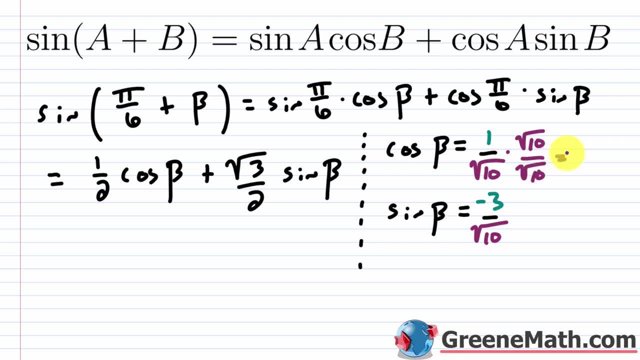 So this is times the square root of ten over the square root of ten. So this equals the square root of ten over ten. And then here times the square root of ten over the square root of ten. So this equals negative three times the square root of ten over ten. 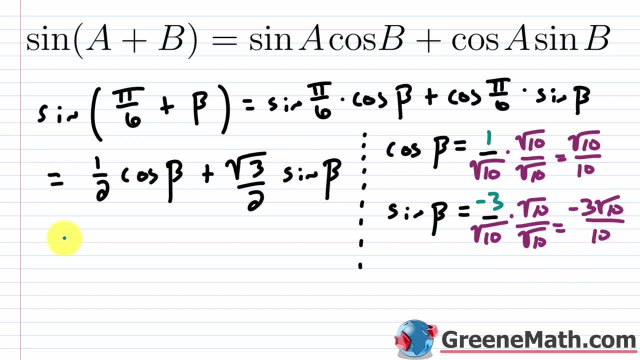 OK, so I just need to replace here and here, So what I'm going to have. let me put equals. You have one half times the cosine of beta is the square root of ten over ten, And then, plus, you have the square root of three over two times the sine of beta. 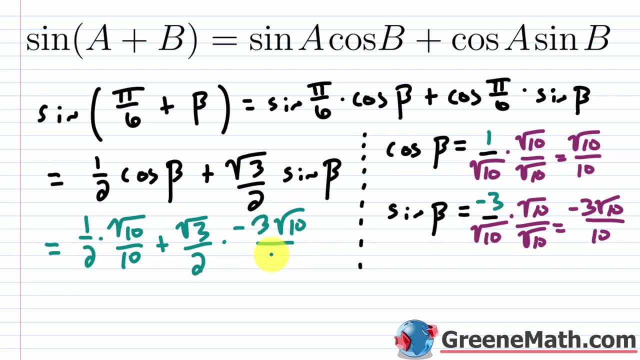 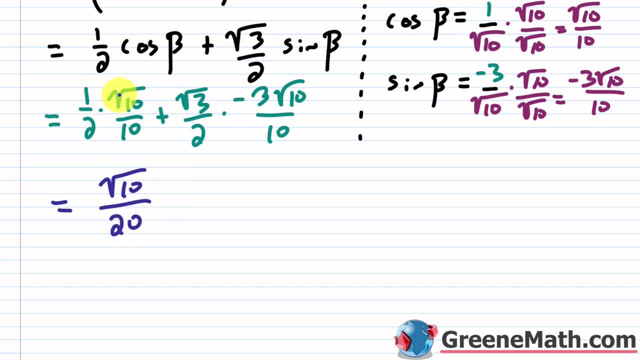 That's negative- three times the square root of ten over ten. So this equals- I would just multiply and say this is the square root of ten over twenty. just multiplying one times the square root of ten, That's square to ten, and two times ten is twenty. 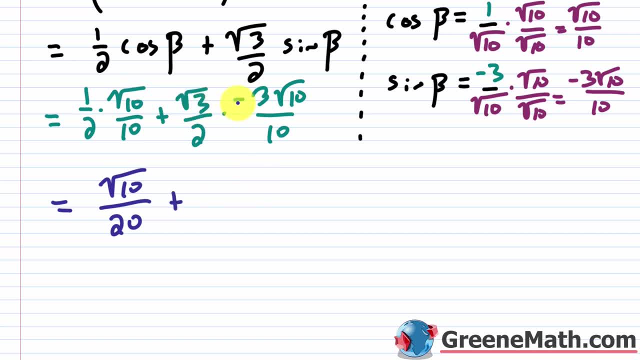 So then you have plus, you have the square to three times negative, three times square to ten. So let's go ahead and write that as a negative here And I'll put three times the square root of thirty. Square to three times square to ten is square to thirty. 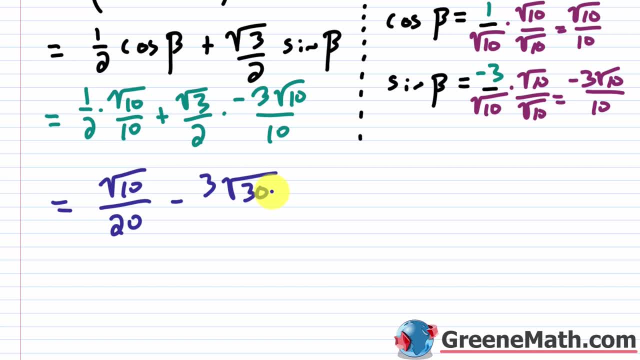 And you really can't simplify that any further, because thirty is six times five, six is two times three, So you really can't do anything more with that. So then this is over two times ten, That's going to be twenty. So what I'm going to do is write this with a common denominator. 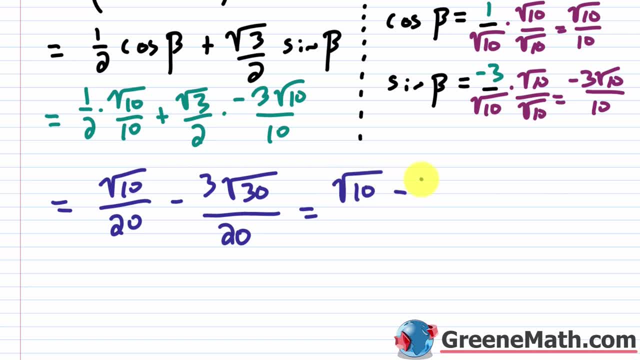 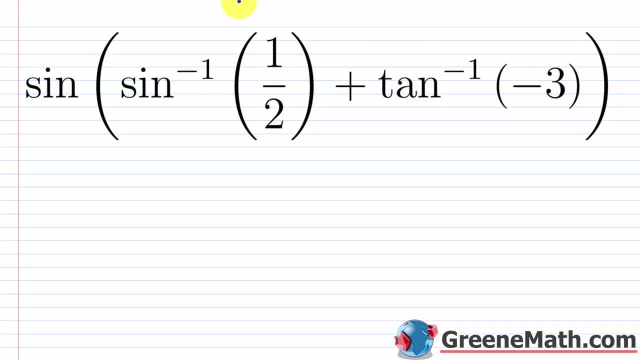 So I'm going to say this is the square root of ten minus three times the square root of thirty over the common denominator of twenty. All right, So let's come back up here to the top And let me just paste this in: So I'm going to say that the sine of the inverse, sine of one half plus the inverse, 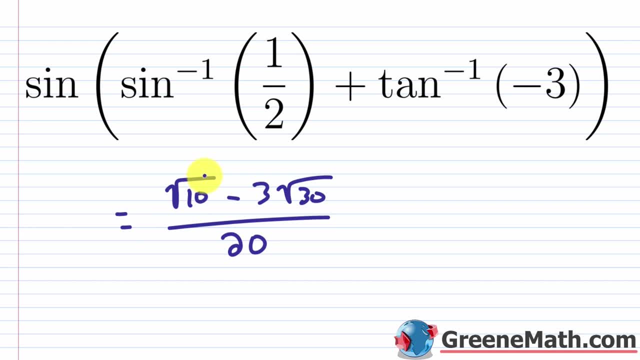 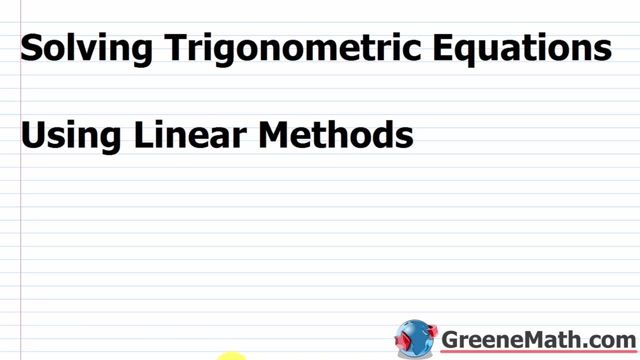 tangent of negative three is going to be equal to this: square to ten minus three times square to thirty over twenty. In this lesson, we want to talk about solving trigonometric equations using linear methods. All right, So let's start off with the easiest possible scenario. 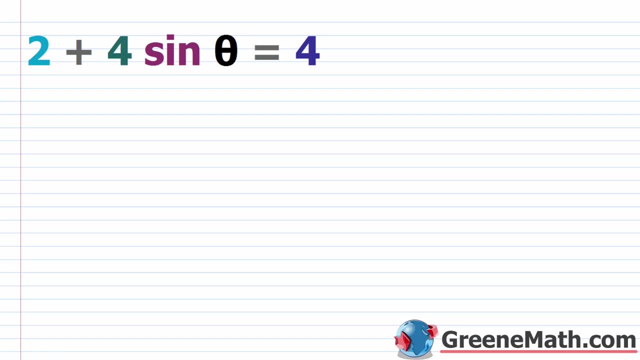 We're going to solve some trigonometric equations again with these linear methods. Let's say you had something like two plus four times the sine of theta is equal to four. So what we're trying to do here we're trying to find values of theta. 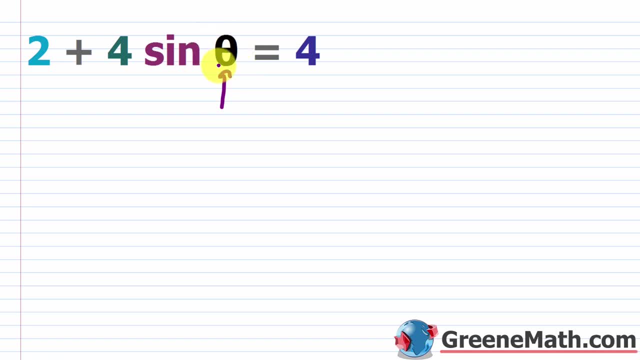 And we're going to try to find the equation that makes the equation true. Now, before I go through this, let's just look at something from basic algebra. So we'll remember this: If I had something like two plus four, x is equal to four. 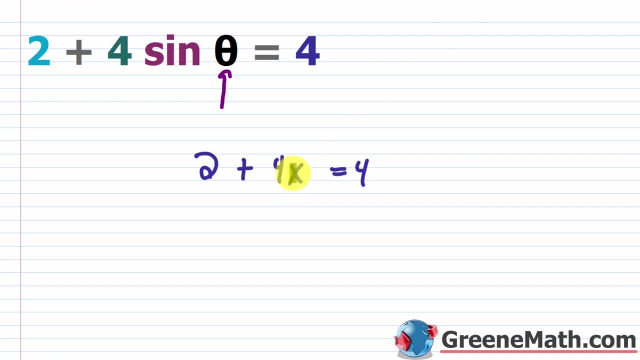 How would I solve this? Well, I'm trying to find values for x that make the equation true, Right? So I would first try to isolate x, So I would subtract two away from each side of the equation, And so this is going to cancel. 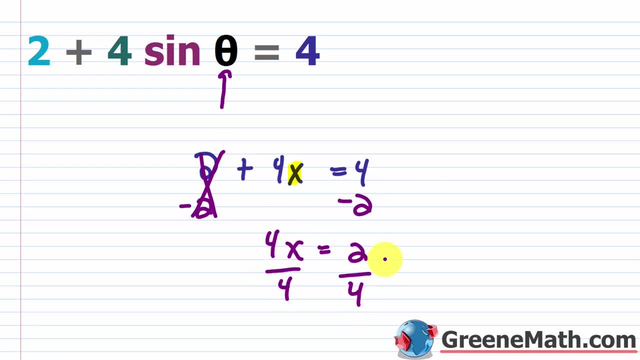 I would say: four x is equal to two. Divide both sides by four And I get that x is equal to one half. OK, so I plug a one half in there and basically have what you have. two plus basically four times a half is two. So two plus two gives me four. 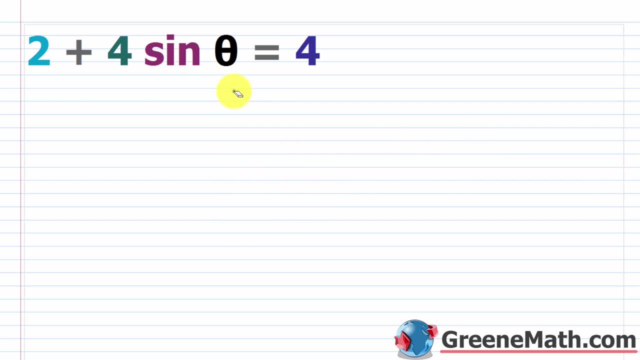 So that is the correct solution. with this guy It's not as straightforward, It's not as easy because, remember, you're plugging in an angle measure there. Sine of that guy would give you a number OK. so you're looking for sine of some value. 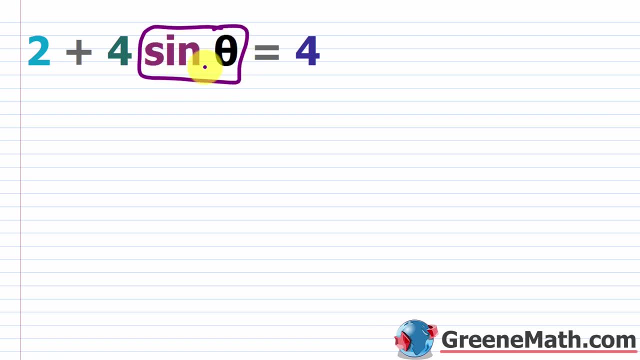 I can already tell you that this needs to be a half for this to be true. So where is sine of theta equal to a half? OK, that's what you're going to be looking for. But to solve this fully, let me subtract two away from each side of the equation. 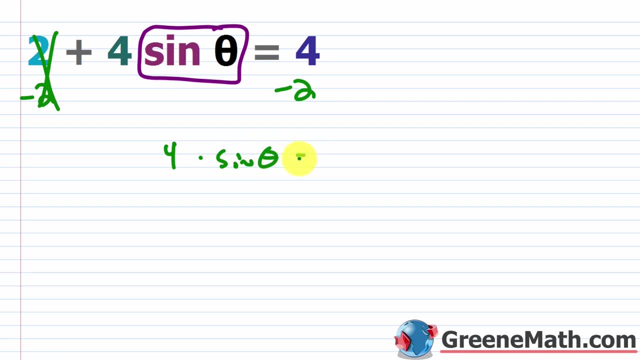 This cancels, We get four times. the sine of theta is equal to two. We divide both sides by four And basically we're going to get that the sine of theta again is equal to a half. OK, so from this guy right here, 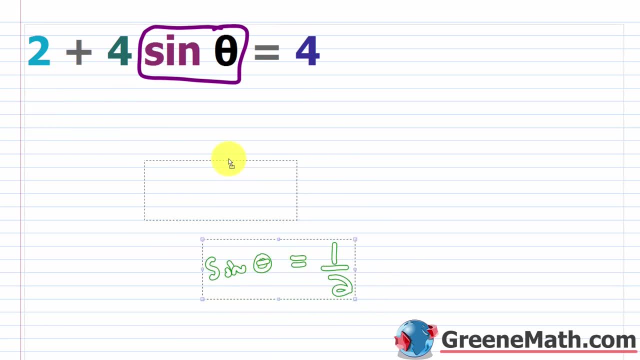 this is where you need to basically do a little bit of detective work. OK, there are so many ways to solve this. It's not even funny. You might want to use a calculator and use the first sine function. You might want to use the unit circle. 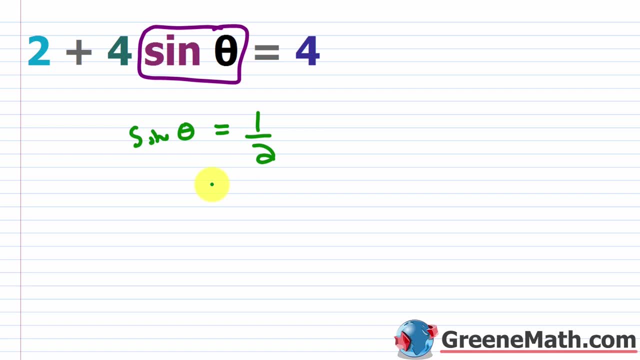 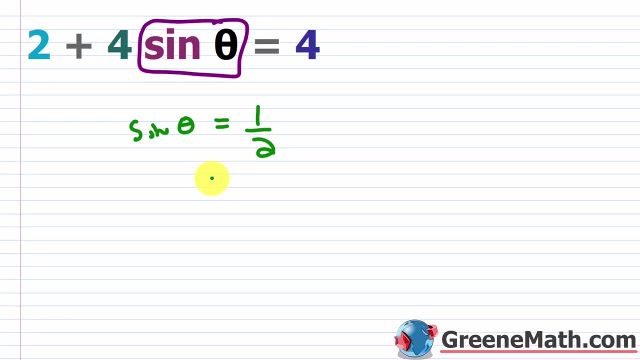 There's a lot of different things that you could do. You could use the special triangles that you remember all kinds of ways. So let me talk about two ways that you can solve this. First, let's think about the unit circle approach. So if you are lucky and you get an easier, 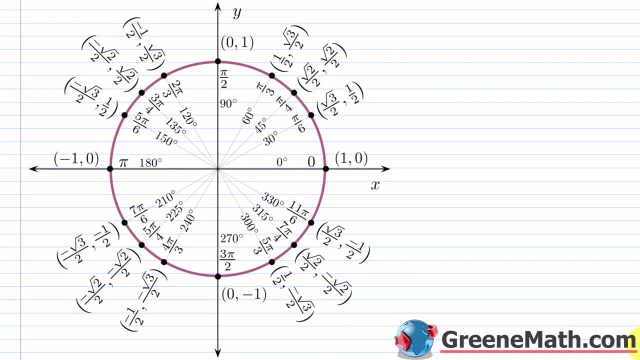 problem where, basically, you can find this from the unit circle. you can go to the unit circle If I'm looking for sine of theta is equal to a half. we can look for the y coordinate and find out where it's a half. OK, so for 30 degrees or pi over six, in terms of radians, the y coordinate is a half. 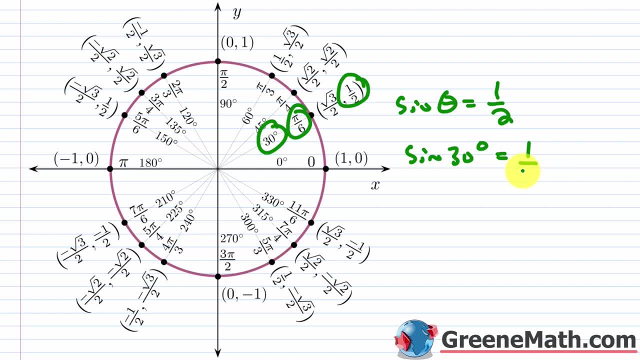 Right. So that tells me that sine of 30 degrees is equal to a half. Then also I know that sine is positive in quadrant two. So remember, when we think about reference angles, if the reference angle is 30 degrees, then sine of that guy is also going to be a half. 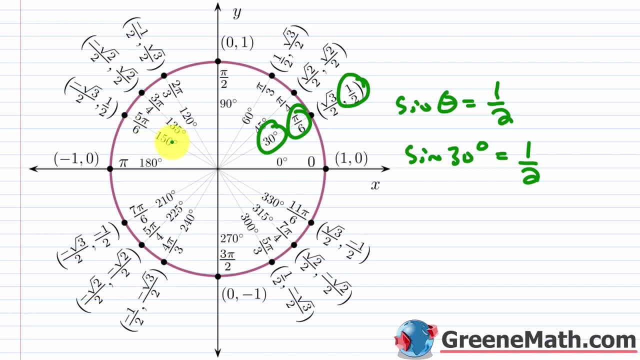 Right. So where would I have a reference angle of 30 degrees? Well, with 150 degrees, right? because 180 degrees minus 150 degrees, the reference angle will be 30 degrees. So, sine of 150 degrees, sine of 150 degrees, and I'm messing up my writing there- 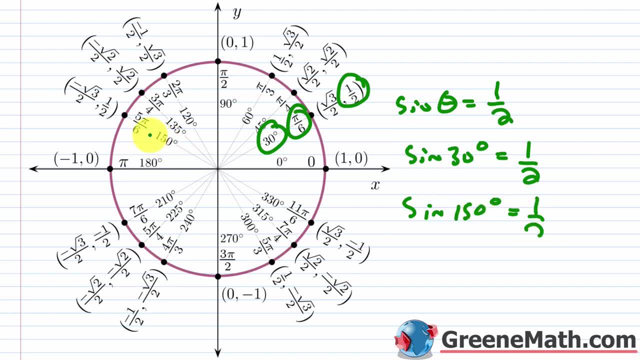 So sine of 150 degrees would also be a half Right, And you can see that here This is a half, This is 150 degrees, or five pi over six if you're talking about radians. Now when you talk about solutions over, 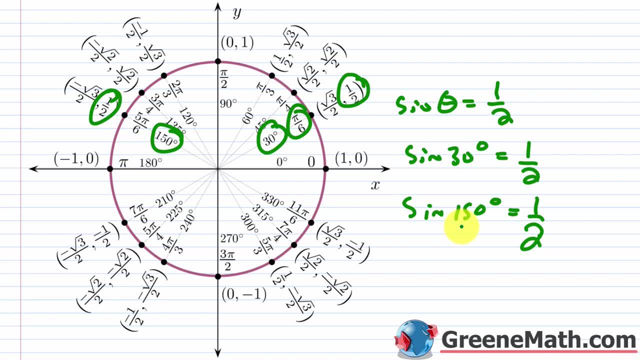 the interval from, if you're thinking about zero, to 360 degrees. your solutions would be 30 degrees and 150 degrees. But when you think about a general solution, remember when you think about sine and cosine, the period is 360 degrees or two pi. 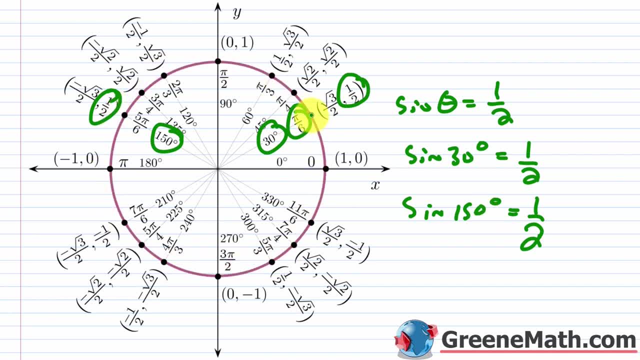 OK. so that means if I started here and I rotated around 360 degrees, well, instead of 30 degrees now I'd have 390 degrees, and sine sine of 390 degrees would also be a half. OK, if I had a 360 degrees again, then sine of in that case. 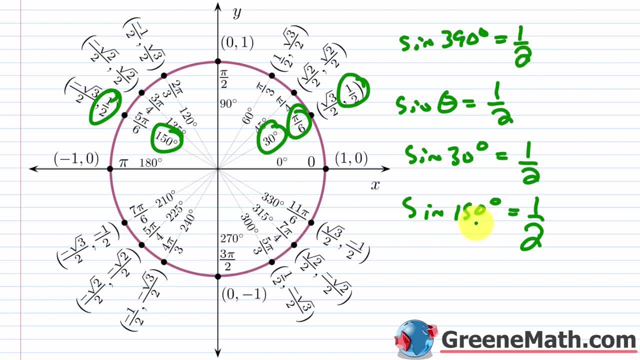 750 degrees would also be a half. you know, so on and so forth. Same thing with 150 degrees. If I had 360 degrees, I'm going to be at 510 degrees. Sine of that guy would be a half as well. 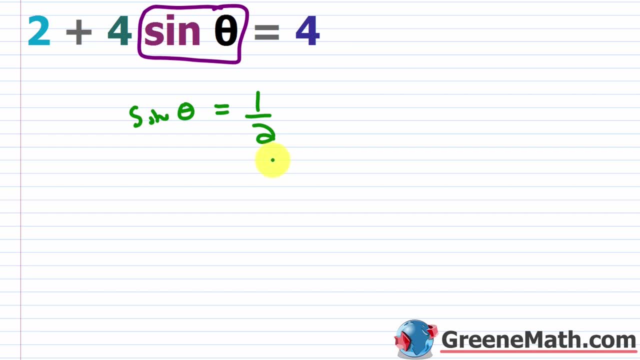 OK, so let's take that information and come back here and give a solution. OK, so first let's pretend we're restricting the domain. So zero to 360 degrees, or again you might see this in terms of radians. So you might see zero to two pi in terms of radians. 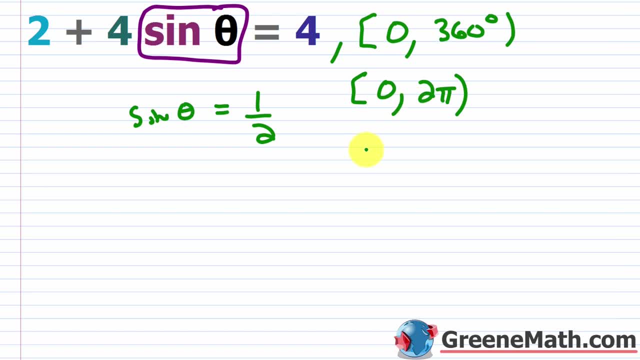 Whatever you get, you want to match that in terms of your answer. OK. so if you get degrees, put degrees. If you get radians, put radians. OK, so in this case I'll just do both. So in this particular case, I'll say that theta is equal to- we had 30. 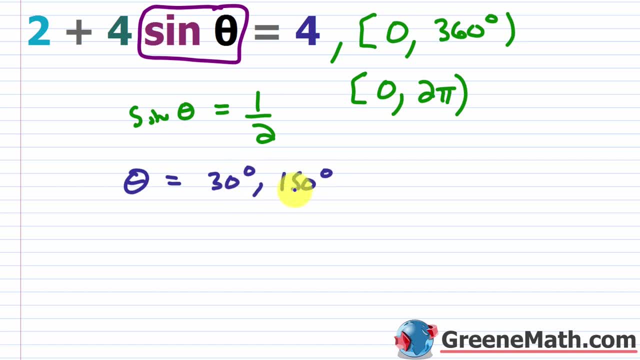 degrees and then also 150 degrees, And again you know the reference angle for both of those going to be 30 degrees. And then, if we look at in terms of radians, we could say theta is equal to pi over six. This is 30 degrees in terms of radians and then five pi over six. 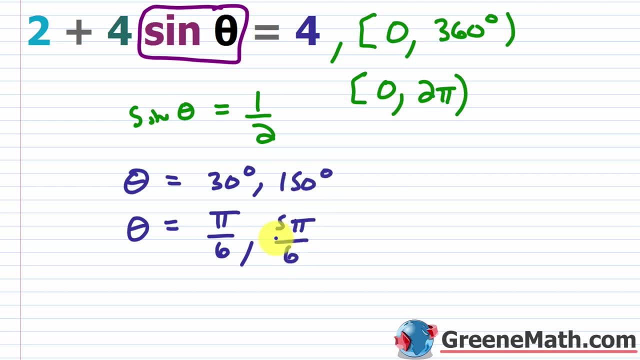 This is 150 degrees in terms of radians. Now, this is the solution for the restricted domain. If you want a general solution, So let me put the general solution OK. so this is going to keep working as we either rotate clockwise or counterclockwise. 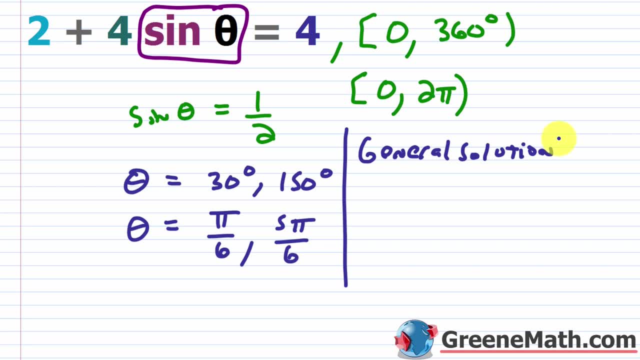 So remember, if you go 360 degrees, it doesn't matter which direction. If you go negative direction, So you're going clockwise, or go the positive direction, So you're going counterclockwise, You're going to keep getting these guys. 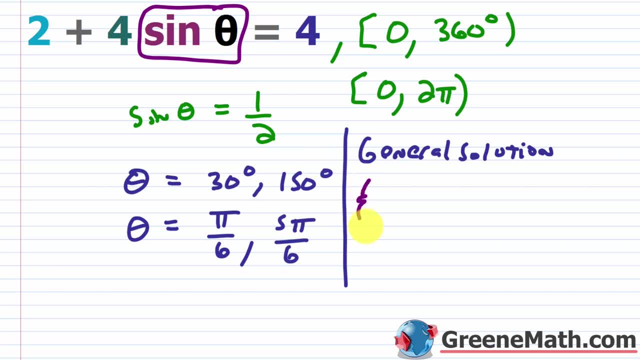 OK, so I'm going to start with, let me make some set braces here. OK, this is typically how you'll see it. I'm going to take this solution. You could do it degrees, or you do radians, I'll do both. So 30 degrees plus the 360 degrees. 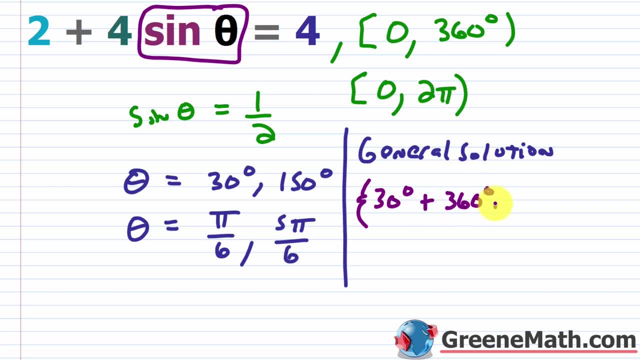 OK, when you go around again, you're going to get that same value, and then times n or n is just any integer, OK, and then I'm going to do 150 degrees and then plus this, 360 degrees. Let me slide all of this down because it's not going to fit. 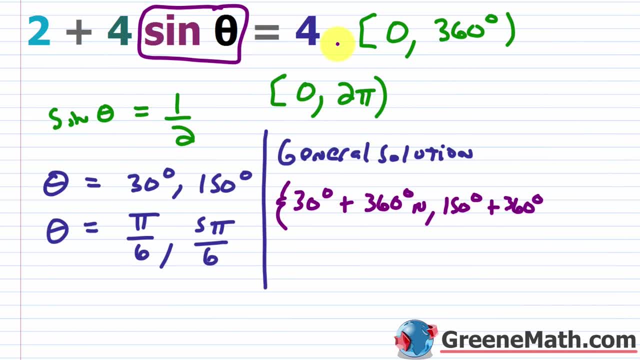 Let me move this down and let me put this comma back where it should be: right there. OK, so this I'll close. my set braces and I forgot my end, So let me put the end there. OK, so that's your general solution in terms of degrees with radians. 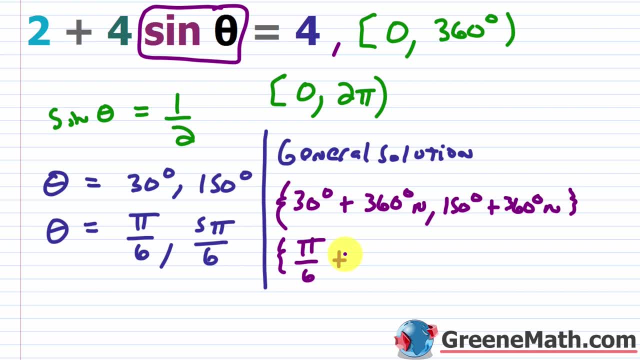 You would say: pi over six plus 360 degrees is just two pi. OK, so I'm going to put two pi n and I'm going to do five pi over six plus two pi n, OK, so there's your general solution. There's your solution for having this domain restriction. 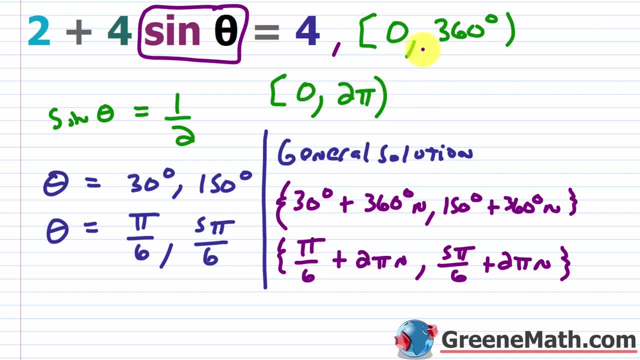 OK, we're basically, you're, between zero and two pi, or, if you think about this in terms of degrees, zero and 360 degrees. Now let's talk about another way that you could have gotten this answer In a lot of cases, especially harder cases, 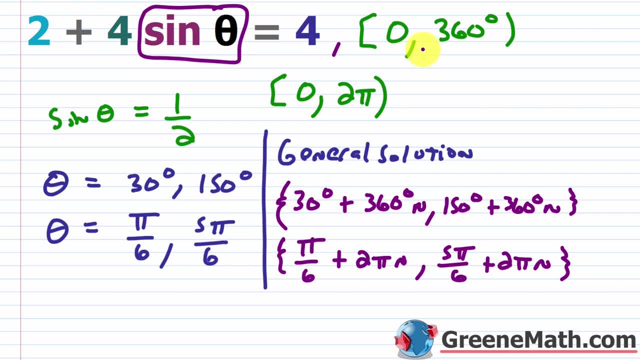 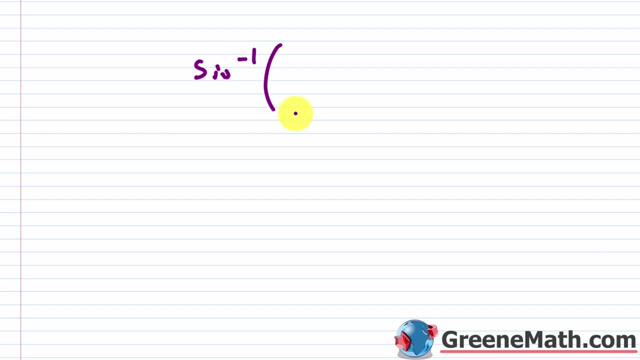 you're not going to be able to use the unit circle. OK, so what you want to do is use your inverse sine function. So let me use a fresh sheet here. Let's say I, I looked on my calculator and I did inverse sine of in this particular case. 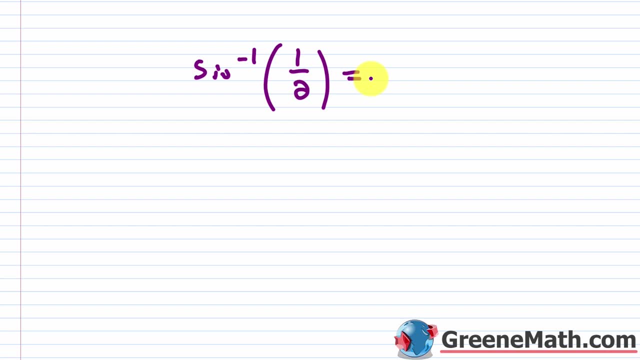 we were looking at a half. OK. so you punch this into your calculator and we already know you're only going to get one value, right. You're just going to get 30 degrees. OK, but again, if I think about sine, of theta is equal to one half. 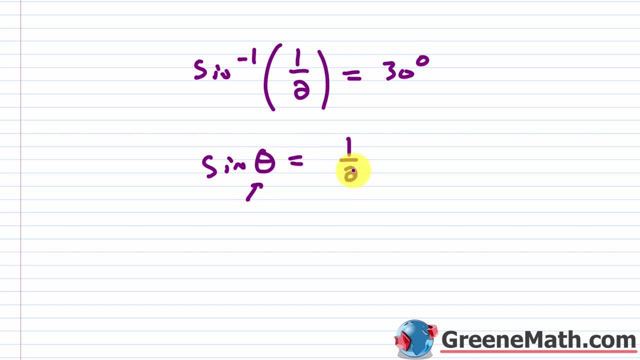 there's an infinite number of angle measures there. that's going to be true for this, and if I have one of them, then I can find all of them again, Because where is sine positive? It's positive in quadrants one and two. 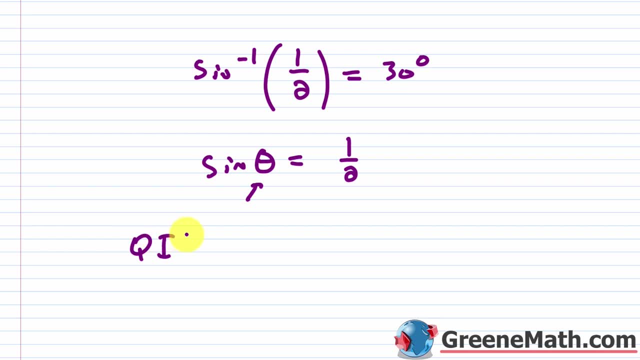 OK, so I have the answer from quadrant one. I have my answer from quadrant one. It's going to be 30 degrees And again it repeats. So 360 degrees in either direction. So if I go plus 360 degrees or if I go minus 360 degrees, 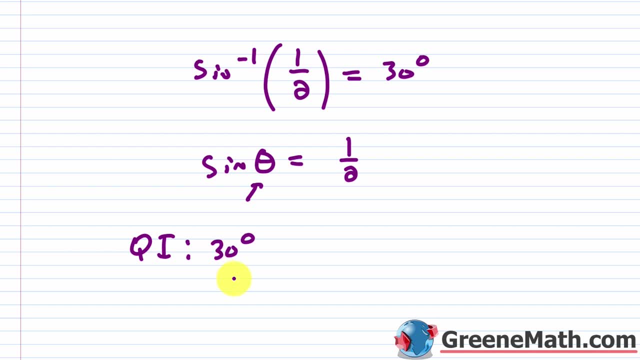 I'm going to again run into another solution, But in quadrant two I just need an angle where the reference angle is 30 degrees, OK. so again, that's going to be found by taking 180 degrees. So I would take 180 degrees, OK, minus 30 degrees. 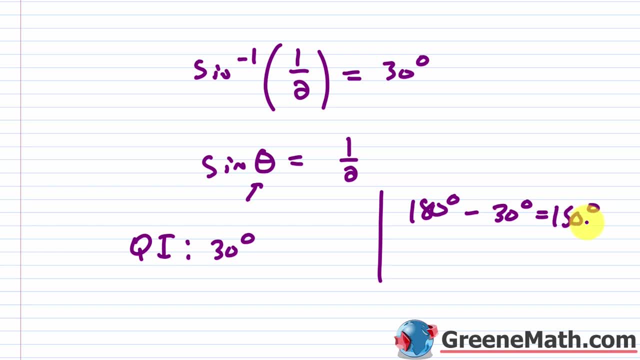 And that gives me 150 degrees. OK, so this is the angle I'm looking for. So in quadrant two I get 150 degrees. So that's another way that you could solve this. You could also use special triangles if you wanted to. 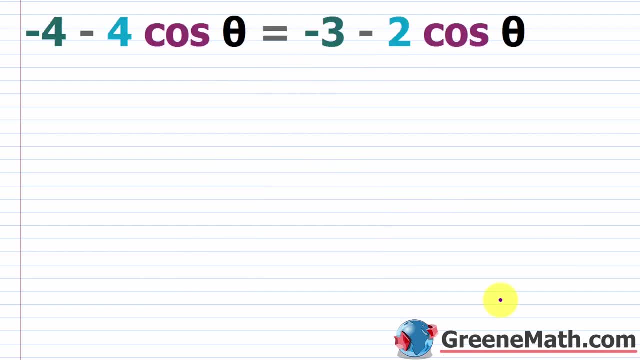 OK, so there's a lot of different ways to think about this guy. OK, let's look at another example. So we have the cosine of theta now instead of the sine of theta. So we have negative four minus four times the cosine of theta, is equal to negative three minus two times the cosine of theta. 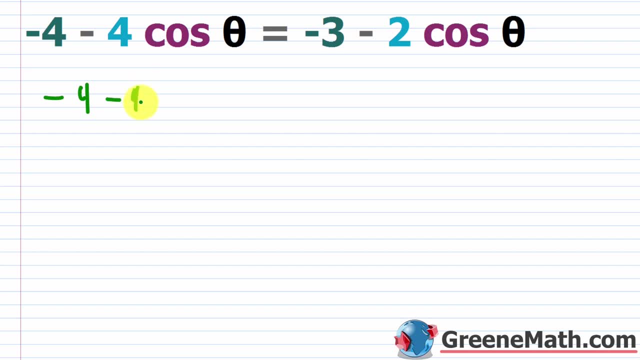 And again, if you are working with this, let's say you had something like negative four minus four X is equal to negative three minus two X. Well, I'd want to get all the terms of X on one side, all the numbers on the other. 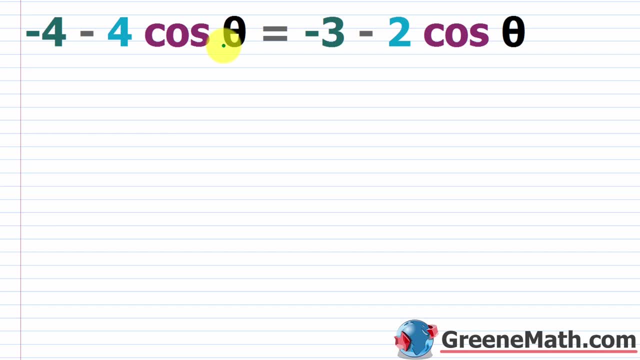 Same thing here. I'm going to get all the terms with cosine of theta involved on one side, all the numbers to the other. So let me add four to both sides, OK, and let me add two cosine theta to both sides, OK. and basically we see that over here this is going to cancel over here. 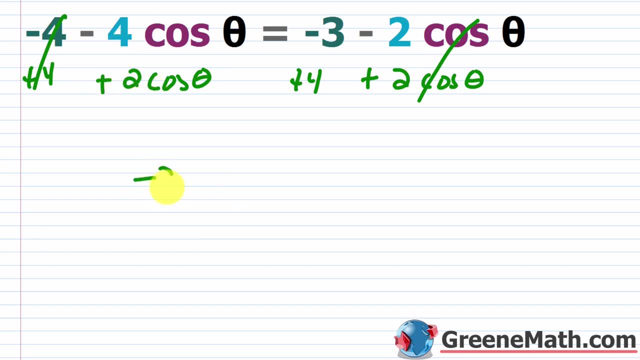 This is going to cancel. So I have negative four plus two, which is negative two times. the cosine of theta Is equal to negative three plus four, which is one. OK, to isolate this guy, I'm going to divide both sides by negative two. 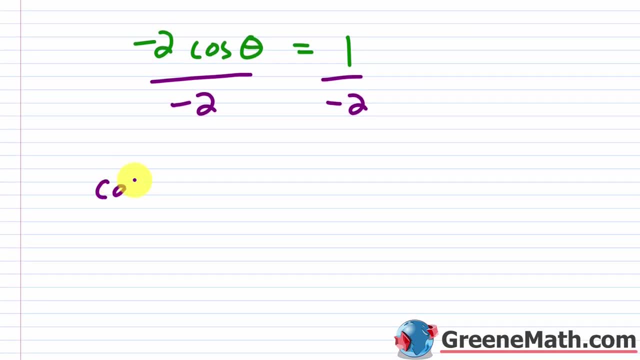 And I'm basically going to find that the cosine of theta is equal to negative one half. Again, another easy problem where you can get this from the unit circle. But let's go ahead and use our inverse cosine function. So let's go: cosine inverse of negative one half. 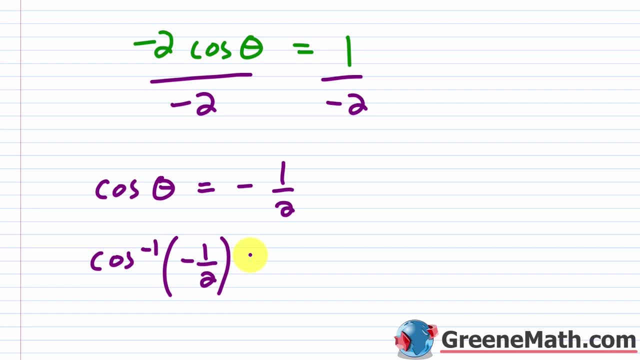 And let's do a little bit of detective work. If you punch that in on a calculator, you're going to get one hundred twenty in terms of degrees, OK, so let me erase this so I can drag this up. We'll have a little bit of room. OK, let me bring this up. 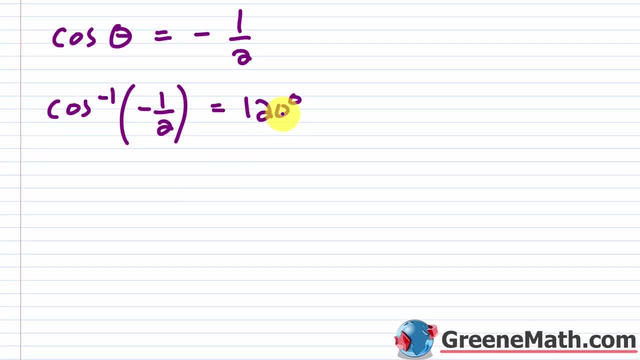 And let's think about this. so I have one hundred twenty degrees there. OK, so in terms of the reference angle, for that, remember, if you're in quadrant two, the reference angle is one hundred eighty degrees minus your angle, which is one. 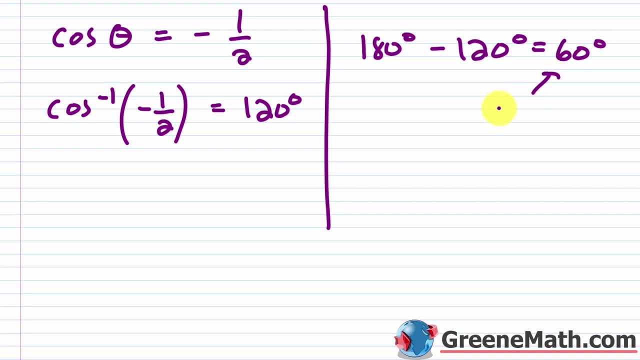 hundred twenty degrees. so this is going to be sixty degrees. So this is my reference angle. OK, so what I want to do now, again, this is negative here. cosine is negative in quadrants two and three. So I have my quadrant two solution. 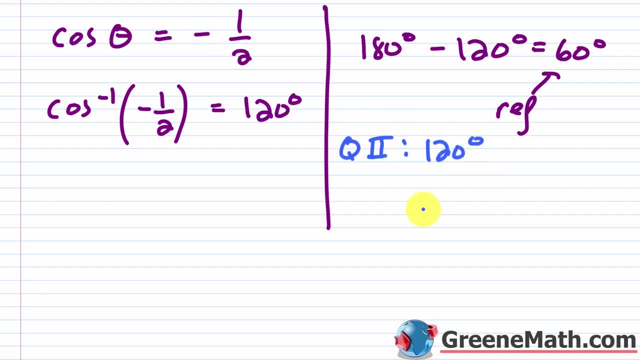 My quadrant two solution is one hundred twenty degrees. for my quadrant three solution, I want to think about an angle in quadrant three. OK, that has a reference angle of sixty degrees. How do I find that? Well, in quadrant three I would want to take one hundred eighty degrees. 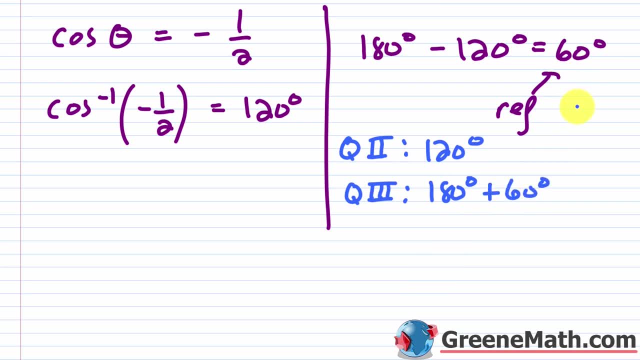 and I would want to add to that sixty degrees, which is my reference angle, OK, which would give me two hundred forty degrees. OK, this is two hundred forty degrees, And the reason that works is, again, if I had a two hundred forty degree angle. 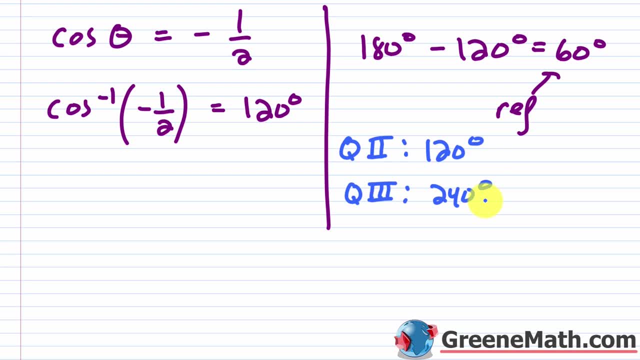 I said: hey, what's the reference angle? You would subtract one hundred eighty degrees to get sixty degrees. OK, so this is my answer in quadrant two. This is my answer in quadrant three. OK, now again, if you wanted a general solution. 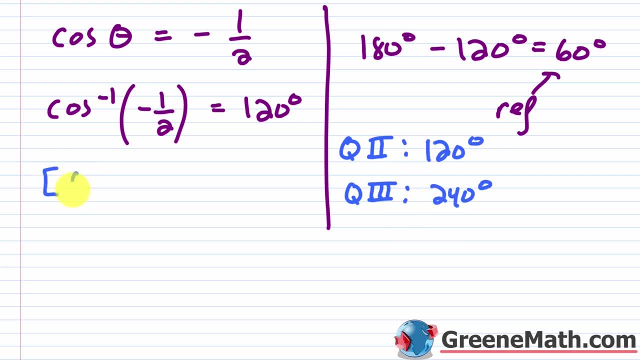 So let's pretend that first you got a domain restriction from zero to three hundred sixty degrees, like this, and then also in terms of radians, we have zero to pi, like this. So for the degrees, you would just put that theta is equal to one hundred twenty. 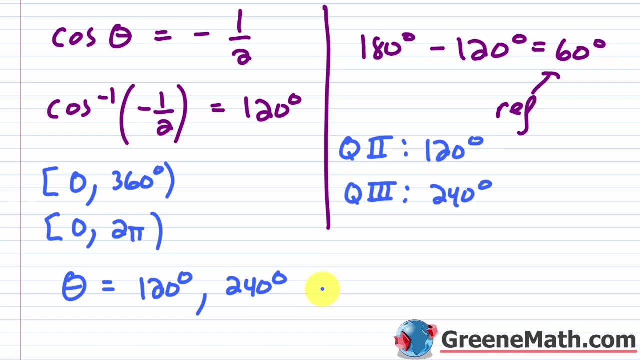 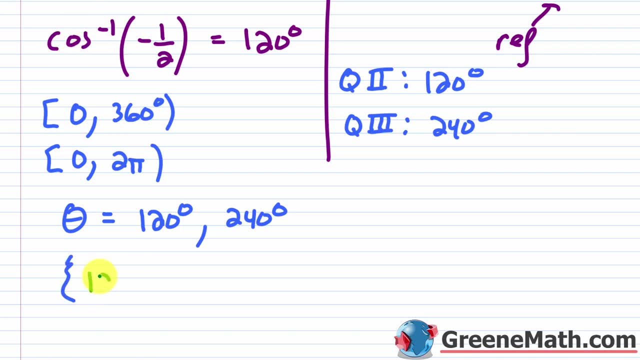 degrees, OK, and then two hundred forty degrees, And then for your general solution. again, all you have to do in this particular case is let's use some set braces here and we'll say: one hundred twenty degrees plus three hundred sixty degrees times n or n is any integer. 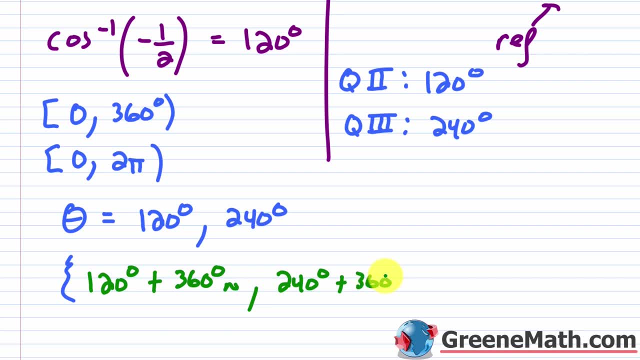 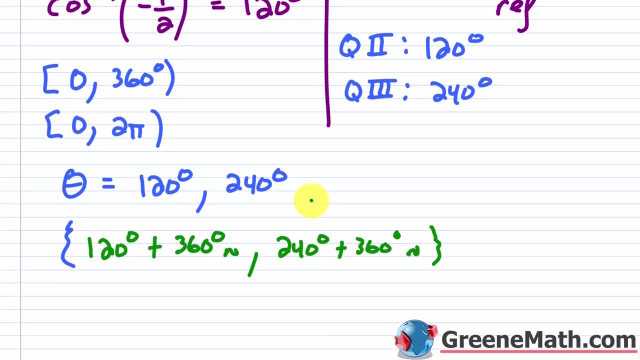 And then you'd have two hundred forty degrees plus three hundred sixty degrees times n or n. is any integer? OK, If you want to do this in terms of radians, we can do that as well, No problem. So we would say something like: theta is equal to within this domain. 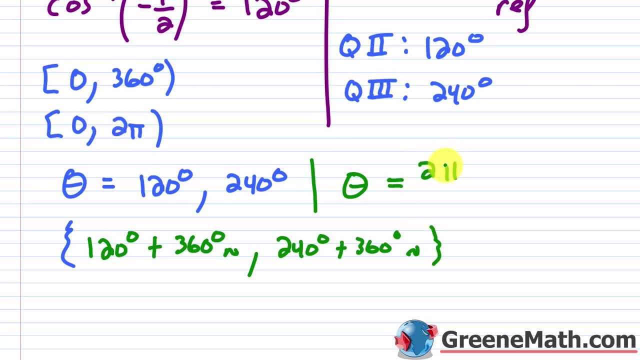 One hundred twenty degrees is going to be two pi over three, OK. And then we also have two hundred forty degrees, which is going to be four pi over three. OK, for the general solution, I just go two pi over three plus two pi n. 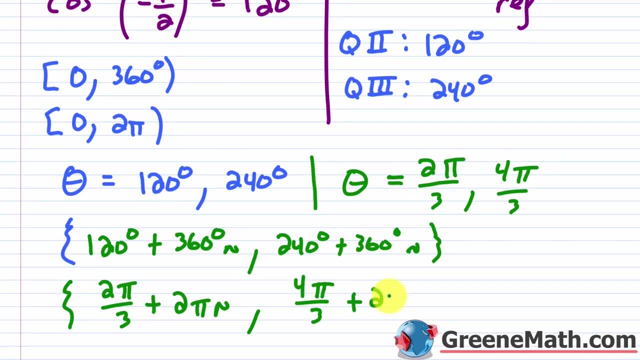 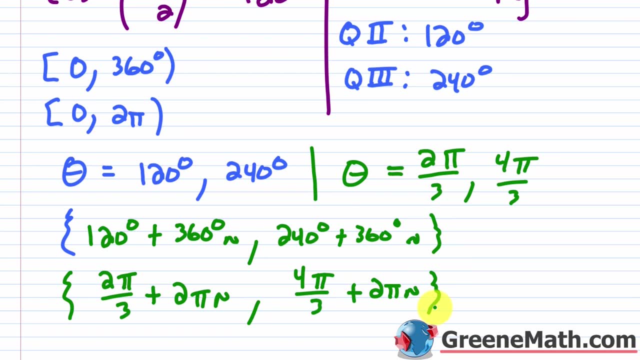 And then I go four pi over three plus two pi n. OK, so again, the period for cosine and sine is three hundred sixty degrees, or two pi in terms of radians. So that's what you want to add. So you have two pi, and then n is just any integer. 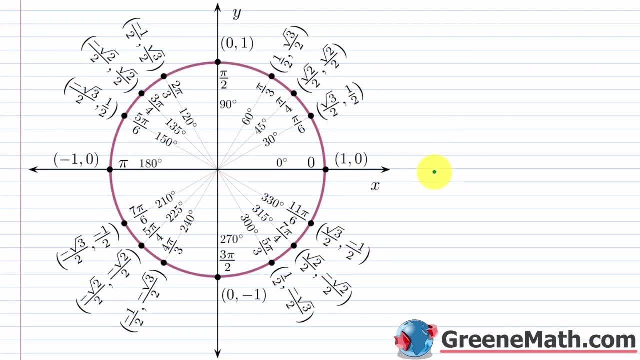 OK, so that's how you want to do that. Now, if you wanted to solve this more quickly, especially if an easy problem, use the unit circle. So where's the X value negative one half? Well, again you come over here. 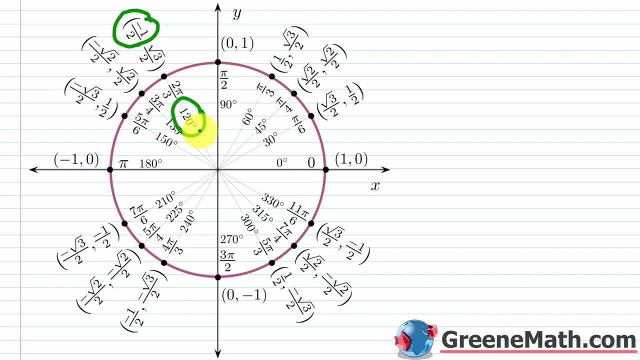 Negative one half is one hundred twenty degrees, or two pi over three radians, OK. and then also two hundred forty degrees pi over three radians. You got negative one half again is the X value, OK, so this is the quickest way to do it. 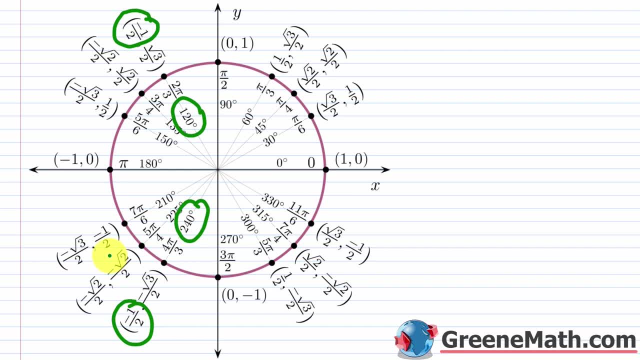 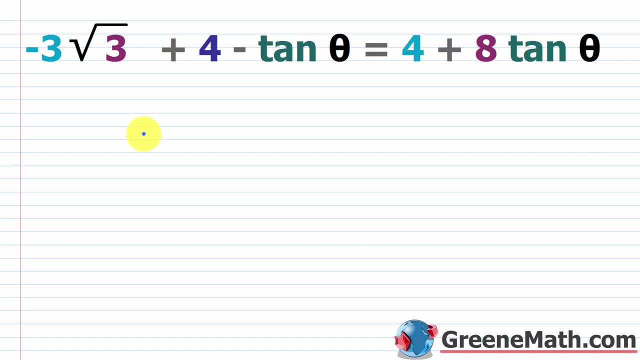 The other way is something you need to understand, because in some situations you're not going to be able to use the unit circle. They're going to at some point give you harder problems. OK, let's look at one more problem, And this one has tangent involved. 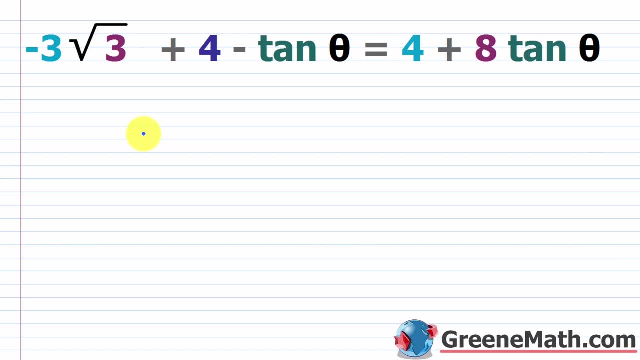 Remember, the period for tangent is now going to be pi or one hundred eighty degrees, So you have to keep that in mind here. So if I have something like the negative of the square root of three plus four minus, the tangent of theta is equal to four plus eight times the tangent of theta. 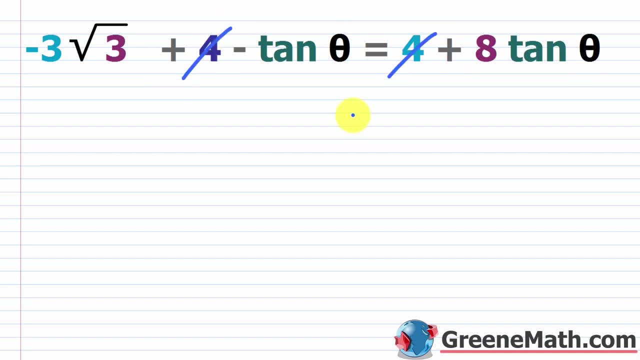 Well, immediately, I can just get rid of the four from each side. Right, Same thing on each side. Just get rid of it. And what I want to do now? let me go ahead and subtract eight times the tangent of theta away from each side of this guy. 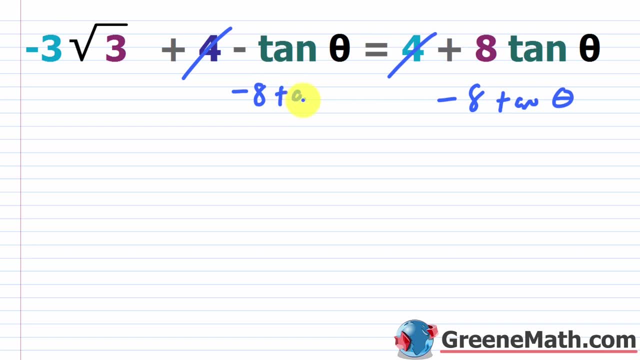 So I forgot my eight. So minus eight times the tangent of theta. OK, so this will cancel out over here. OK, and I'm just going to add three times square root of three to both sides. So what I'm going to end up with is you put a negative one there. 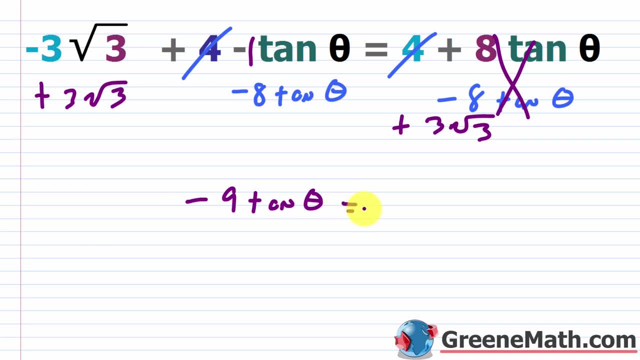 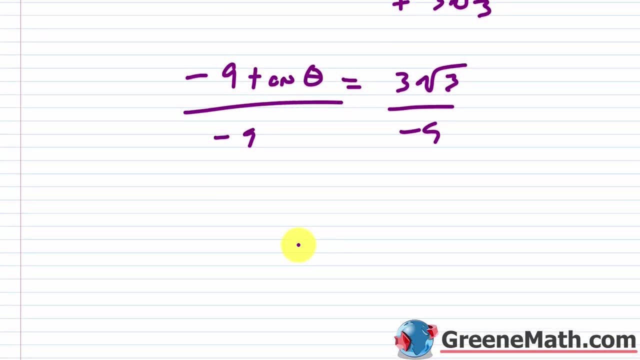 You'll say you have negative nine times the tangent of theta is equal to three times square root of three. Divide both sides by negative nine. OK, let me scroll down just a little bit And I'll say that I have the tangent of theta is equal to the three is going: 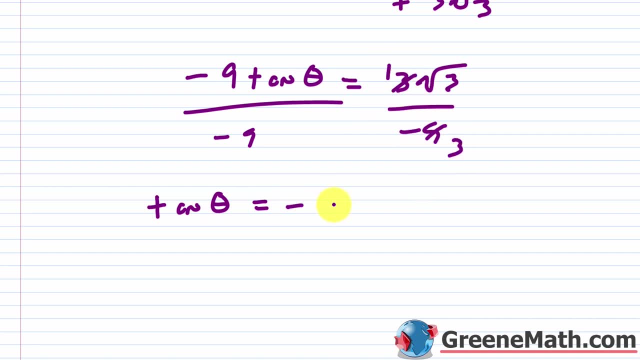 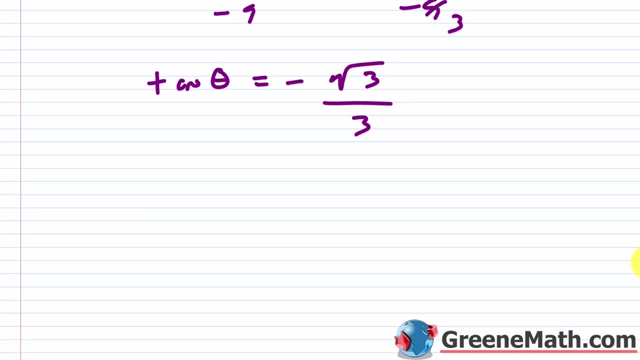 to cancel with the nine. This is a one, This is a three, So let's say the negative of the square root of three over three. OK, so now with tangent, it is a little bit more challenging to think about these. You could. 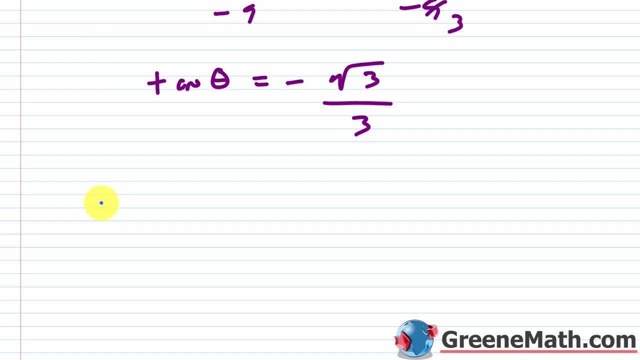 You could use your special triangles in this particular case and just think about the square root of three over three. The tangent of 30 degrees is square root of three over three. So let me just write this over here: The tangent of 30 degrees is equal to the square root of three over three. 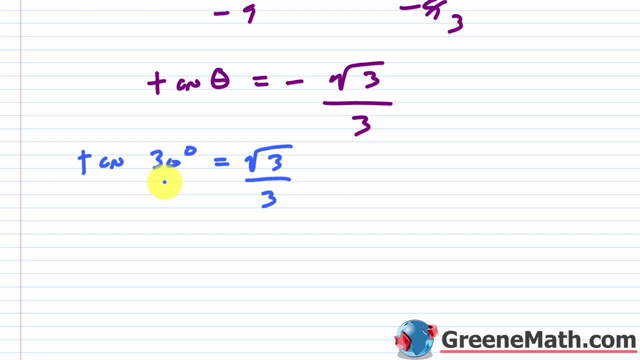 So again, I would say that tangent is going to be negative. Let me draw this out here so we remember this, So we remember the. all students take calculus. So tangent is negative in quadrants four and two. OK, so let's think about this in quadrant two. 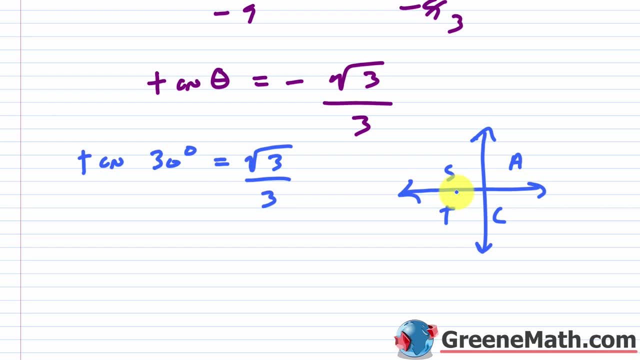 Where would I have a 30 degree reference angle? Again, if I take 180 degrees and I subtract off 30 degrees, that gives me 150 degrees. OK, my reference angle here for 150 degree angle would be 30 degrees. 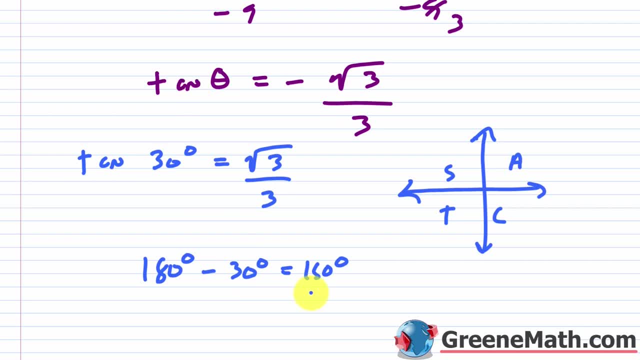 So my value here: if I did tangent of 150 degrees, because it's negative, I would get the negative square root of three over three. OK, so let me erase this for a second. Let me just put one answer here. So theta here. 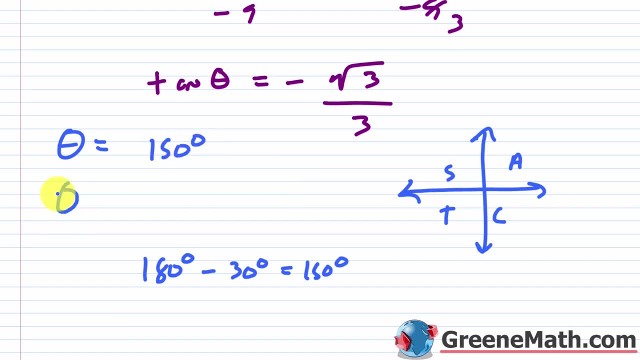 Would be 150 degrees, Or again, if you want to write this in terms of radians, this is five pi over six. OK, whatever you want to do, So let me erase this. for a second. Let's think about in quadrant four. 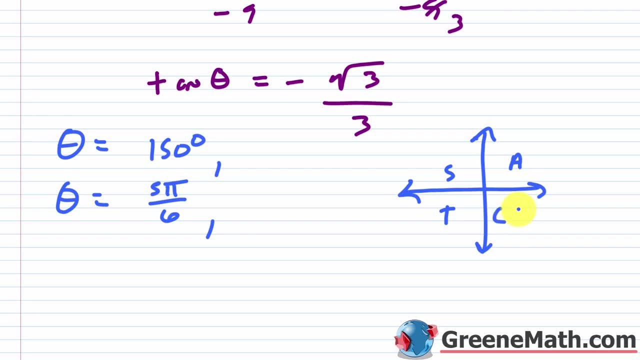 So remember I said the period when you work with tangent is 180 degrees, So I can just add 180 degrees to this, OK, so 150 degrees plus 180 degrees is going to be 330 degrees. OK, also what you could have done. 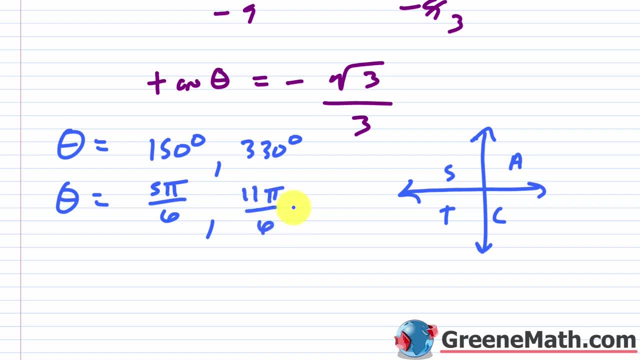 And this is 11 pi over six in terms of radians. Also, what you could have done is again look for a 30 degree reference angle in quadrant four. So in quadrant four I would just go: 360 degrees minus 30 degrees is going to give me 330 degrees. 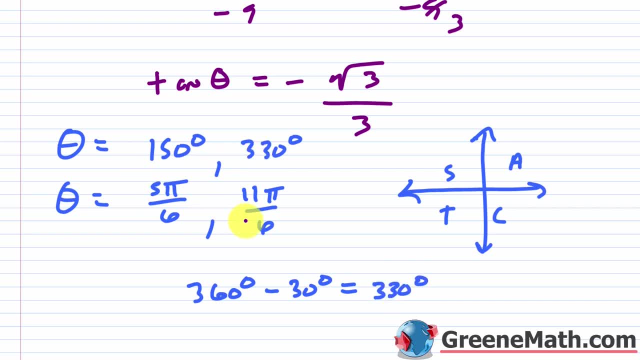 So this is the angle I'm looking for, All right, So obviously these would be your solutions. if you had a domain restriction, OK, but if you didn't have a domain restriction, let me just write this over here. So this is zero to 360 degrees. 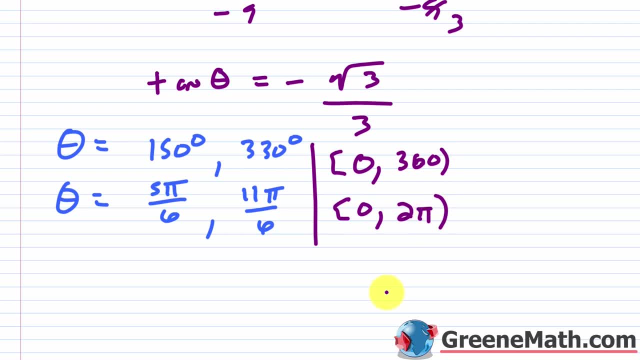 And this one is zero to two pi in terms of radians. If you didn't have a domain restriction. you have to be careful because a lot of students will come through here. They're used to working with sine and cosine, So they go 150 degrees plus 360 degrees times. 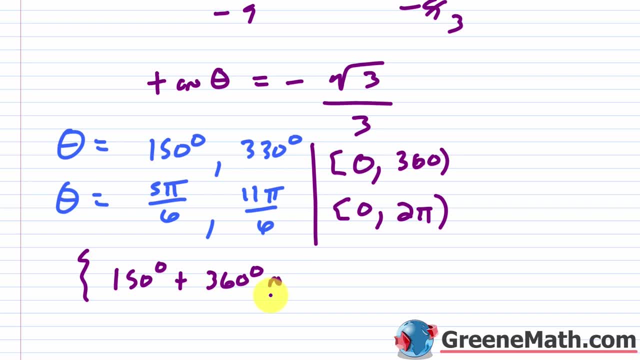 OK, this is actually wrong. OK, the period for tangent is 180 degrees, So you want to put 180 degrees like this. Now do you need to list 330 degrees plus 180 degrees times that? No, you do not. 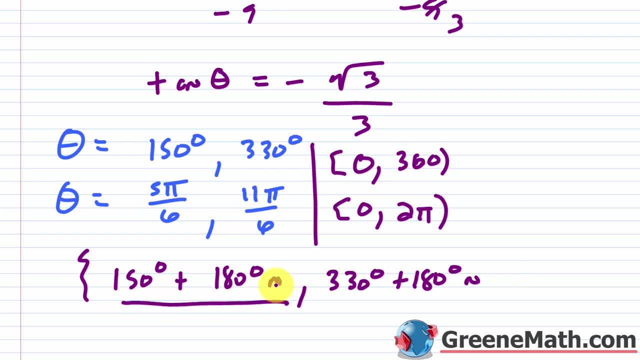 And the reason for this is, if you go back to this one right here, let's say n is one, Well, you're basically adding 150 degrees to 180 degrees, You get to 330 degrees. So you don't need to put this guy in here. 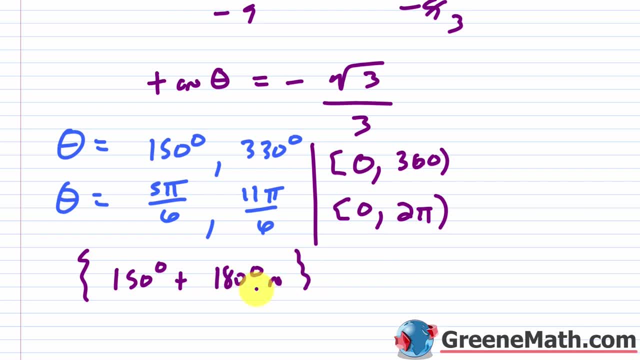 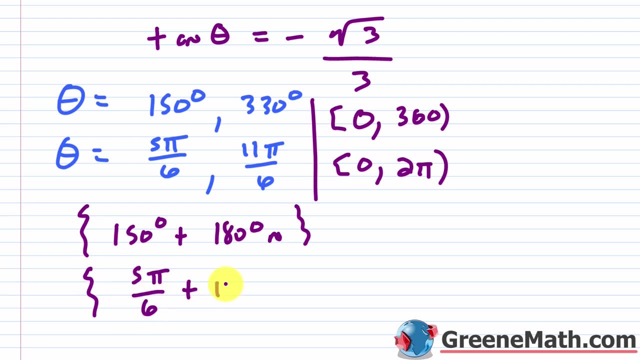 It's just overkill. You just put it like this and be done with it. OK. then the other one over here for radians. you're just going to put five pi over six plus you're going to do pi OK, which is 180 degrees in terms of radians times that. 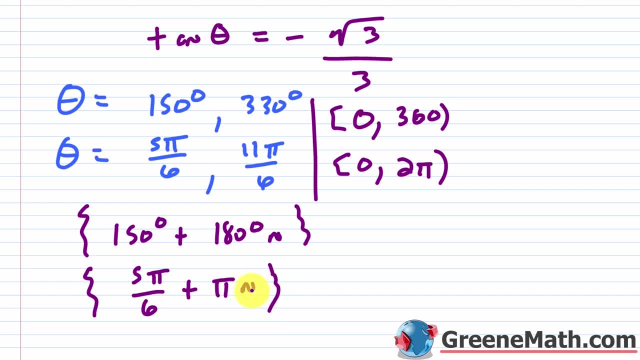 OK, that's all you need to do, because again, if you added basically one, you get a common denominator says six over six. So if you had six pi over six plus five pi over six, you would get eleven pi over six. 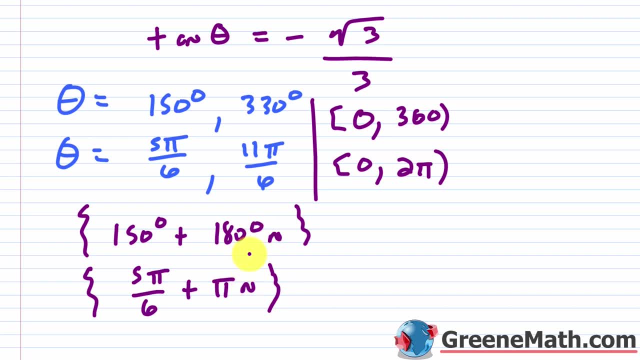 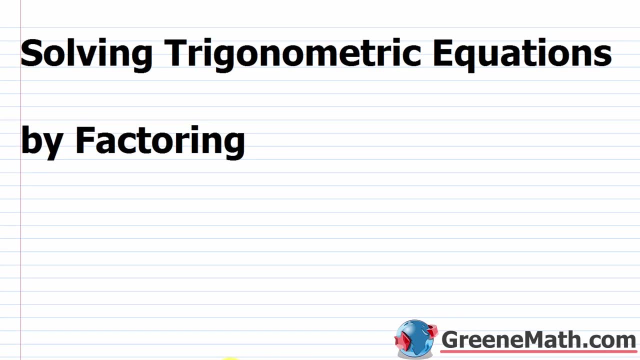 OK, so again, it's overkill to list both of them. in that case, You just want to list it like this, as simply as you possibly can. In this lesson, we want to talk about solving trigonometric equations by factoring. 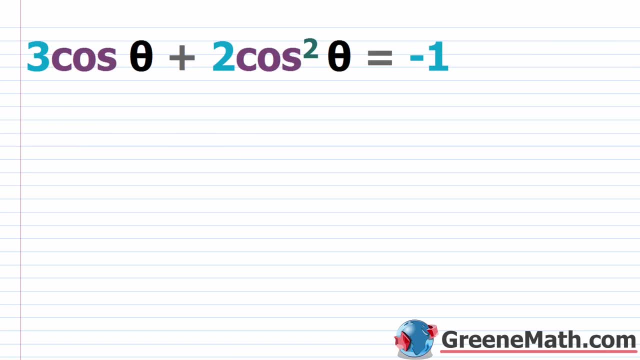 All right. So now we're just going to look at the next scenario. We already talked about how to solve these basic trigonometric equations using linear methods. Now we're just going to be factoring. So we have three times cosine theta plus two times cosine squared theta equals negative one. 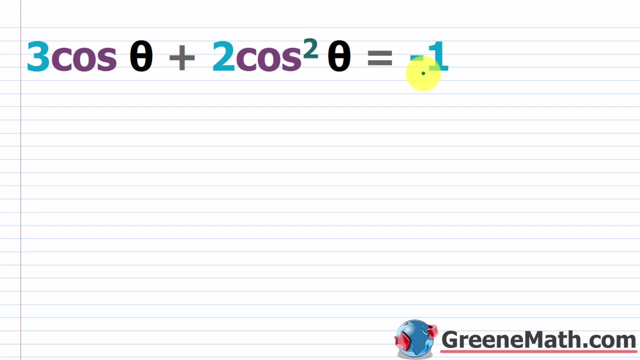 So a very easy problem. You want to get this. If you see something with a squared term in it, you want to think about factoring right away- That's usually how you're going to solve that- And you want to think about getting it in the form of AX squared plus BX plus C equals zero. 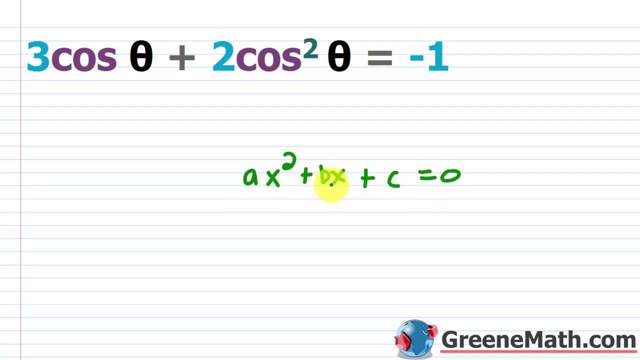 Remember, this is a quadratic and you're able to solve this by factoring and then setting each factor equal to zero. That's the zero factor property. So I'm going to do the same thing here. I'm going to move this to the left, basically. 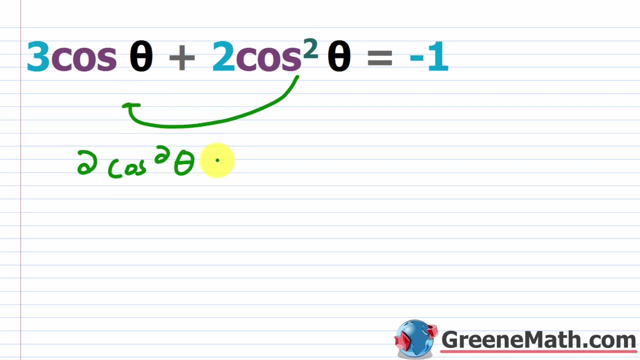 So I'm going to say I have two times cosine squared theta and then plus this three times cosine of theta And I can add one to both sides of the equation. So say plus one in this equals zero. So if I can factor the left side again, I can use that zero factor property. 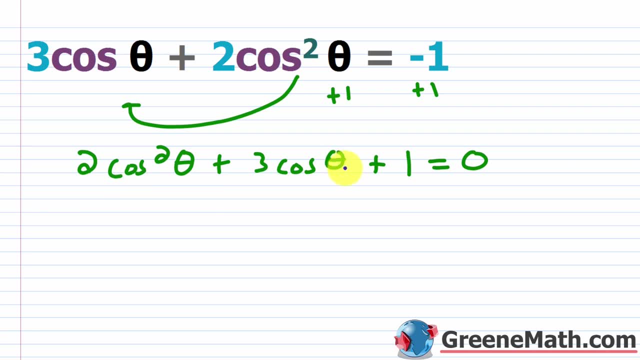 There is a tremendous roadblock to factoring this when you first start. I don't know why it is, but when I work with students- and I'm just going to do it on the first one- I tell them: just make a little substitution. 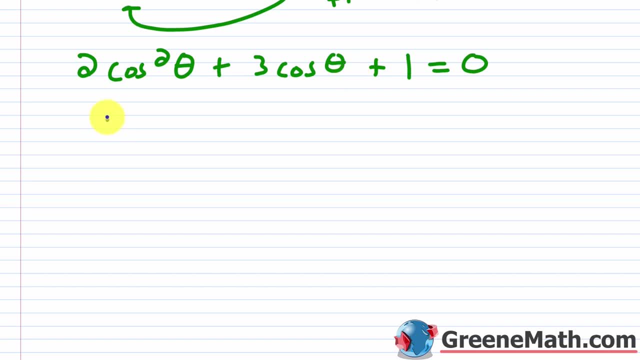 So in this case you're working with cosine of theta, So just let something like you be equal to the cosine of theta. OK, so everywhere you see cosine of theta, replace it with you. So here I have cosine squared theta, which is basically cosine of theta squared. 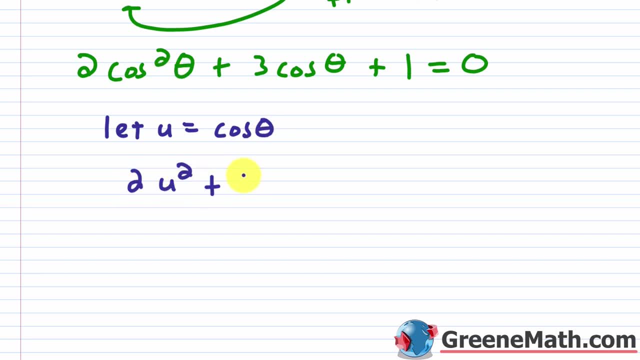 So I would say I have two u squared plus, in this case, three u, and then plus one equals zero. So from here, could I factor this and solve it using factoring? Yes, of course I could. So this guy is a prime number and this guy is one. 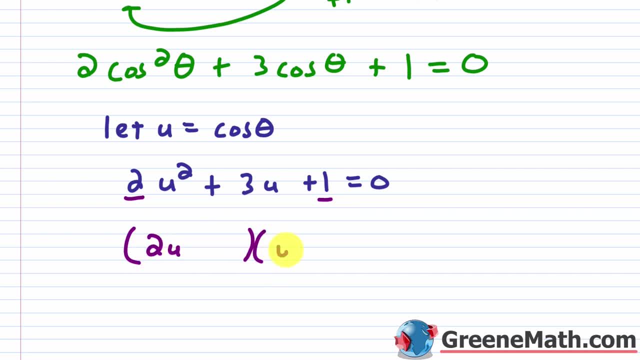 So this is really easy to factor: This is going to be two, u and this is going to be u. We know that off the top and we know that, because this is positive one and all the sines are positive, the only possibility is that this would be one and this would be one. 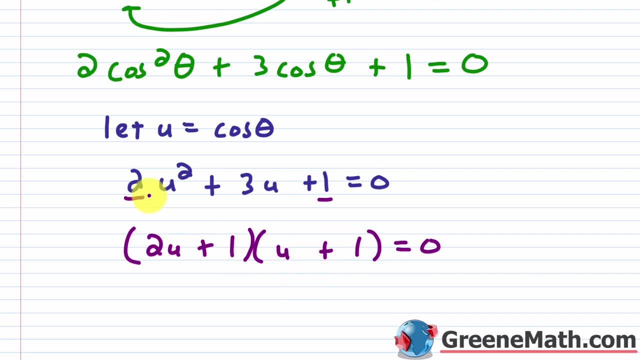 So basically, you would check this and say: OK, well, two u times u is two u squared. The outer would be two u, the inner would be u. So those combined together would give me the three u and the last would be one times one, which is one. 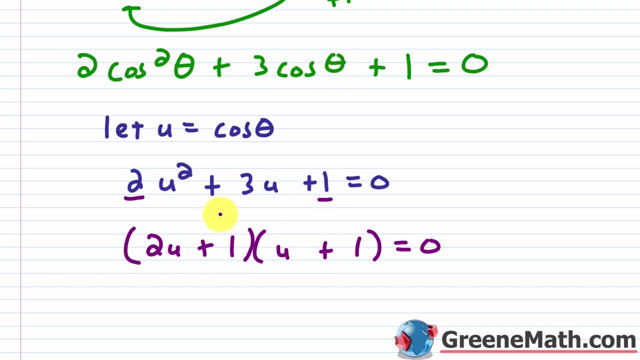 So we're good to go. So you could have factored this the same way, using the same principles, with the cosine of theta in there. But again, I use u there just to avoid the little roadblock of first factoring a trigonometric expression like this. 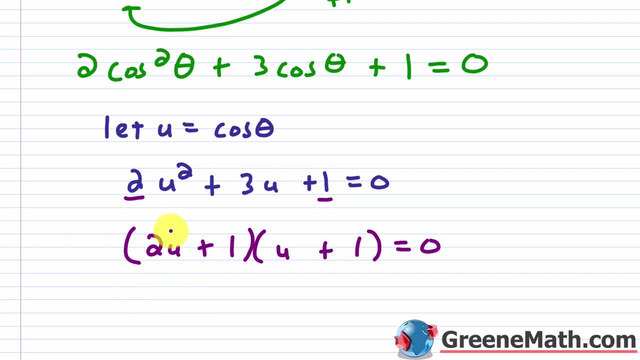 So what I want to do now is, because u is cosine of theta, I just want to plug back in. So I'm going to say two times: everywhere there's a, u I'm plugging in a cosine of theta, then plus one. 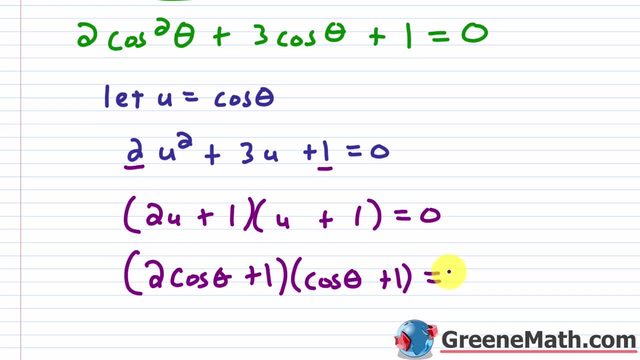 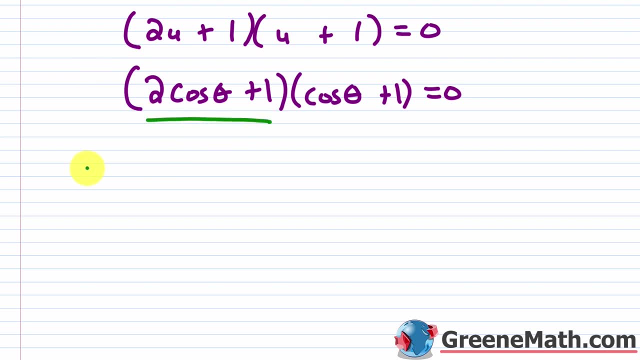 And then times, you have your cosine of theta plus one, and this equals zero. So now that we've got this guy factored, let's set each factor equal to zero and let's see if we can get a solution. So I'm going to start with this one. 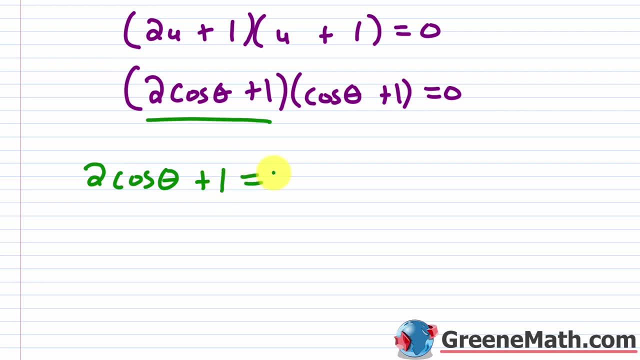 I'm going to say two times cosine of theta plus one equals zero. Let's subtract one away from each side of the equation. We're going to get two times cosine of theta is equal to negative one. divide both sides by two And I'm going to get that the cosine of theta is equal to negative one half. 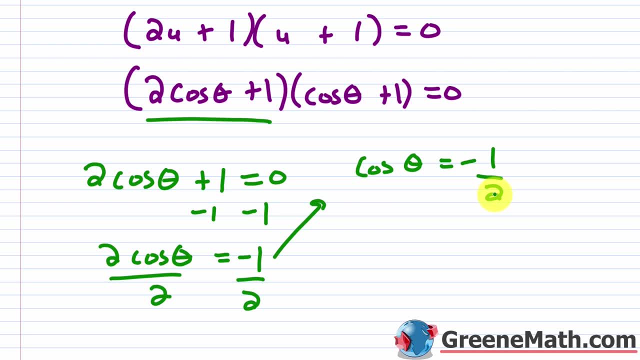 So you're going to see the same numbers pop up over and over again. You probably, at this point, know that the values for this in terms of degrees would be 120 degrees and 240 degrees, but I'll go to the unit circle in a moment and show you. 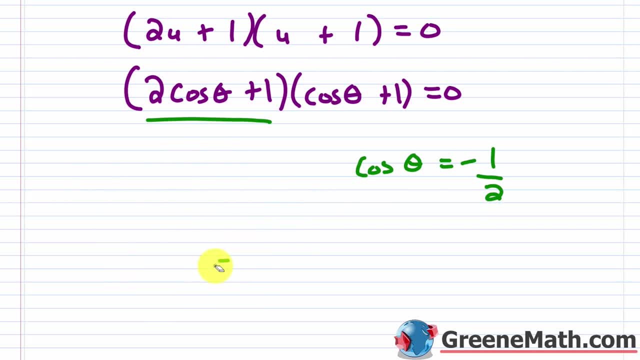 So let me just erase this kind of make this a little bit more neat, And I'll just say that cosine of theta is equal to negative one half. Let me just slide this over Just a little bit And I'll delete this from here. 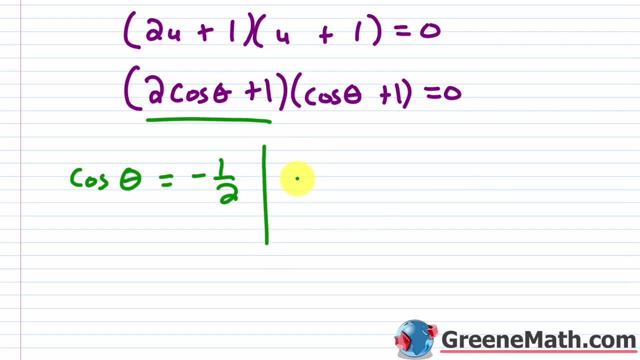 And I'm going to go down to the unit circle all at once. So let's do this side now. So we have cosine of theta. Basically, you're just subtracting one away from each side. So let's, let's do the full thing. 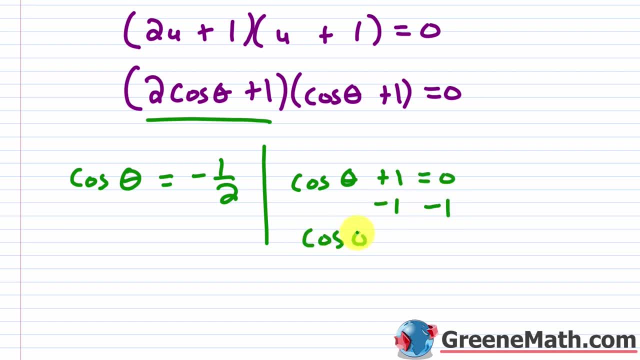 So plus one equals zero. Subtract one away from each side, You get: cosine of theta is equal to negative one. You probably know already this happens at 180 degrees or pi everything at our ratings. So let's move this up and say we have: cosine of theta is equal to negative one. 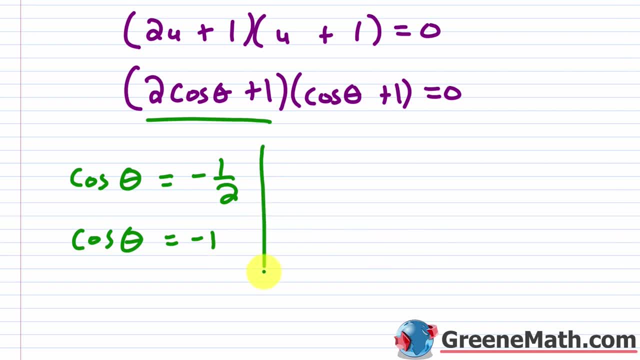 So let's go to the unit circle real quick and get all of our solutions Again. you can also do this using your calculator. You can do it with special triangles. There's so many ways to do it, But for the first two they're very easy. 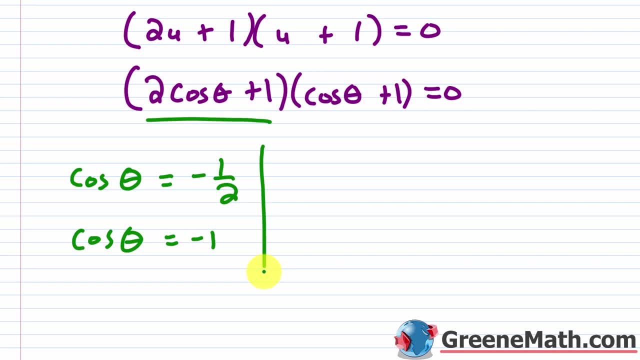 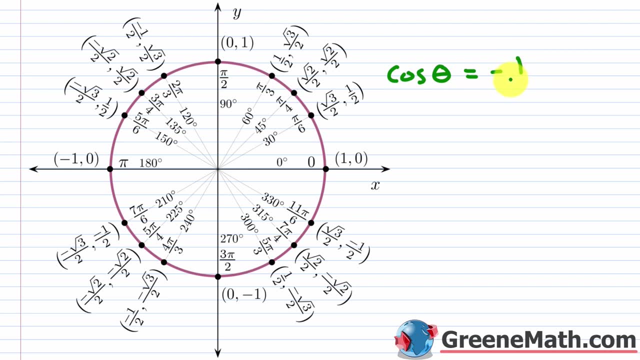 I'm going to give you a final problem where you have to use your calculator. There's no other choice. OK, so we'll see. So let's go down to the unit circle. So again, if we're looking for cosine of theta is equal to negative one half. 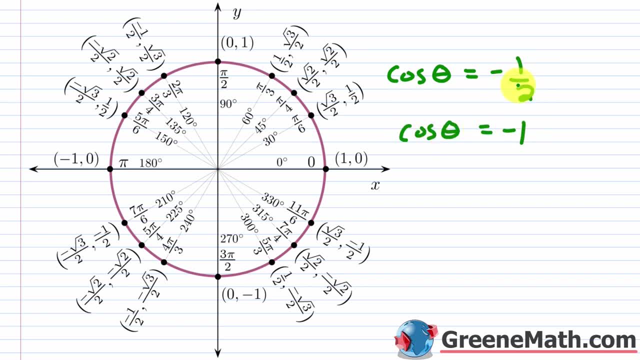 and then cosine of theta is equal to negative one, where you're looking for an X value of negative one half. So that's going to happen here again at 120 degrees, or two pi over three radians. And then also remember this guy would have a reference angle of 60. 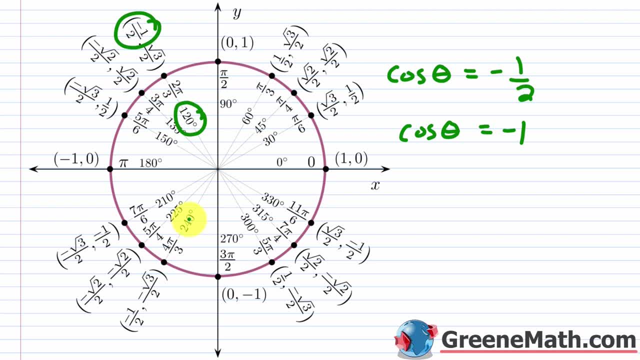 degrees. so you would want 240 degrees because that also has a reference angle of 60 degrees. So this is your negative one, half there, Again 240 degrees, or four pi over three radians. So let's write 120 degrees and then I'm going to write 240 degrees out here. 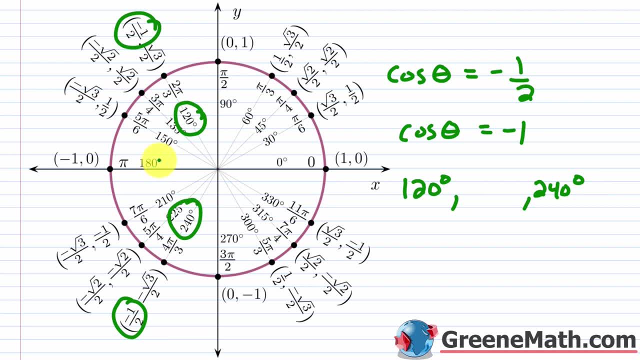 I'll put a little space here, because I'm going to put this hundred eighty degrees here for the negative one, Right? So negative one is your X value there. So let's put one hundred eighty degrees there and let's just put the radians in. 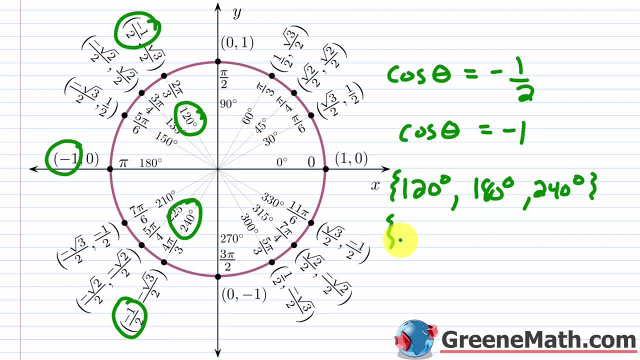 there as well. Generally, you're going to give your answer based on the restriction you get Right. If they tell you the intervals between zero and 360 degrees, you put degrees. If they tell you zero to two pi, you put your radians. 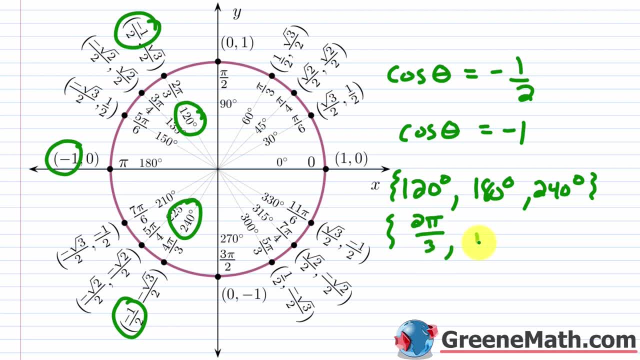 So let's go ahead and put: we have two pi over three, We have pi, and then we have four pi over three. So let's go ahead and copy this. We're going to need that And we're back here, So let me just go ahead and paste this in. bring this over here. 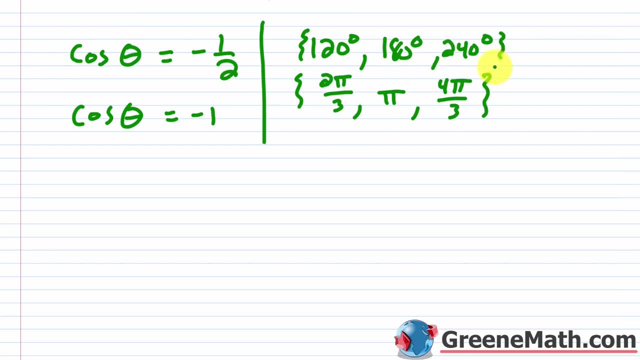 So this is going to be our solution, Again, if you restrict the domain. so for this one, let's say that we restrict the domain from zero degrees to three hundred sixty degrees. OK, so basically in that interval, for this one, this is going to be if you restrict it from zero to two pi in terms of radians. 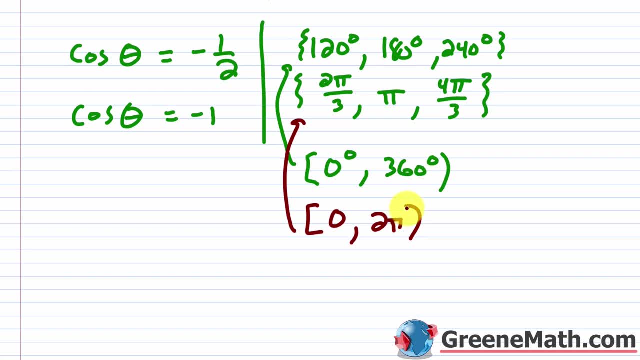 So, based on what you get, that's how you're going to get your answer. If you're asked to get a general solution, remember these guys are going to repeat Right. So with the sine or cosine, if you're working with one of those, the period is going to be three hundred sixty. 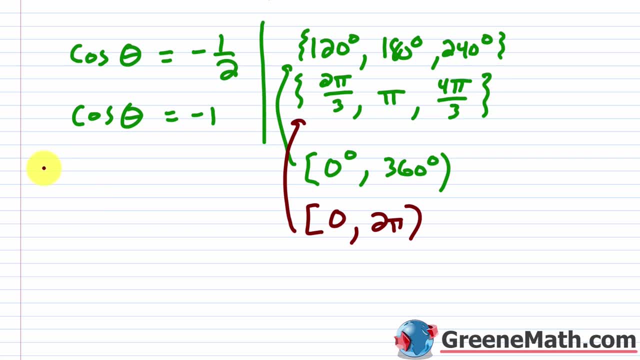 degrees or two pi in terms of radians, So just take this. if you wanted a general solution, So let's put general solution here- You would take these guys. So I'm going to say one hundred twenty degrees plus three hundred sixty degrees times n or n is just any integer. You're just going to take all of them. 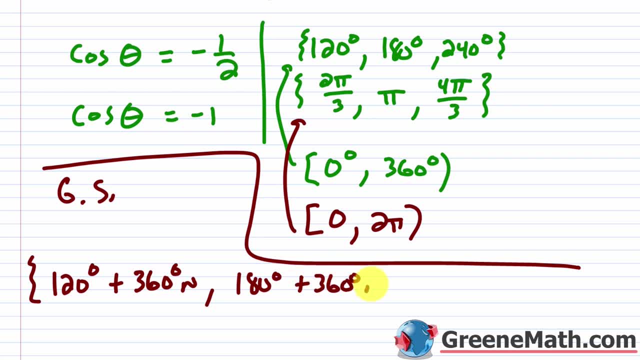 So then, one hundred eighty degrees plus three hundred sixty degrees times n, And then, lastly, two hundred forty degrees plus three hundred sixty degrees times n. OK, let me close the separations. Then, for this one, remember, three hundred sixty degrees is like two pi. 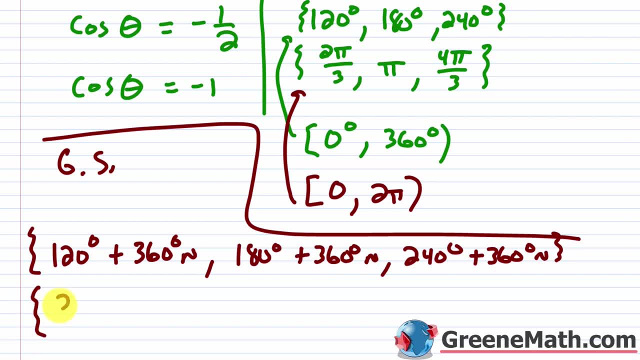 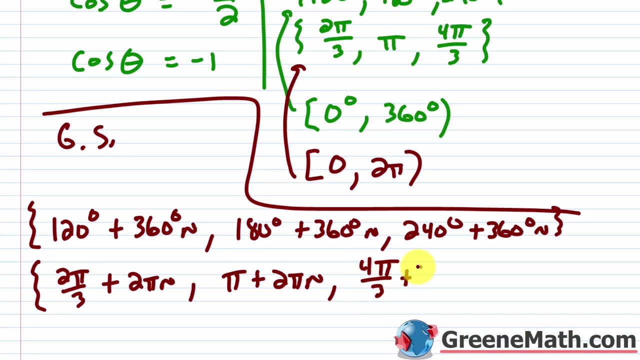 In terms of radians. So what I want to do here is, say two pi over three, and then plus we'll have two pi times n. OK, so n is any integer Same thing. So pi plus two pi n. And then lastly four pi over three plus two pi n. 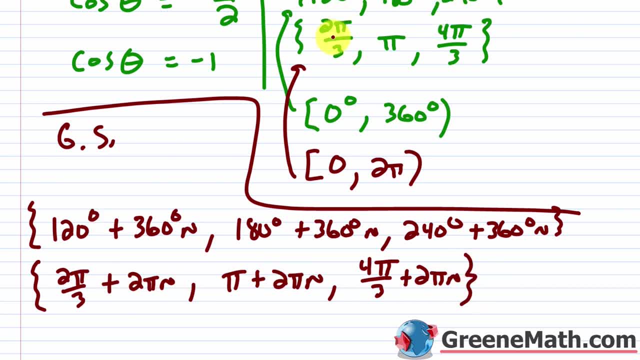 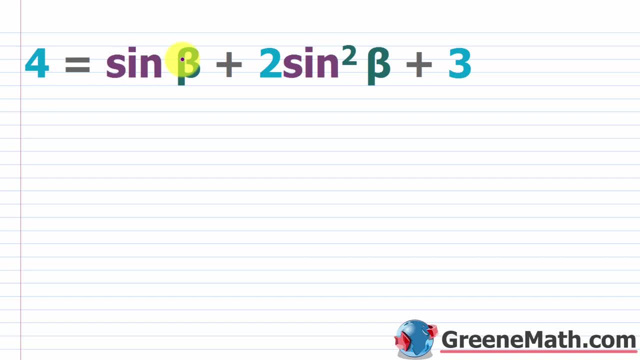 So we have our general solution here and then we have our solution where, basically, we're in an interval. You could say you're restricting the domain. All right, For the next one let's look at four equals: sine of beta plus two times sine squared beta plus three. 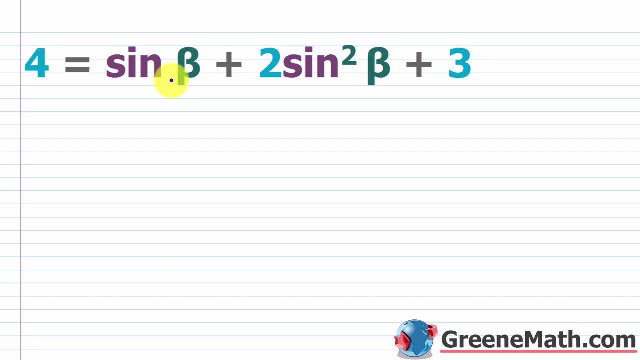 Again, if you have something squared and then something to the first power, I'm always thinking factoring right. I'm always thinking AX squared plus BX plus C equals zero. So I'm going to write it like that. I'm going to first, let's go ahead and flip the sides. 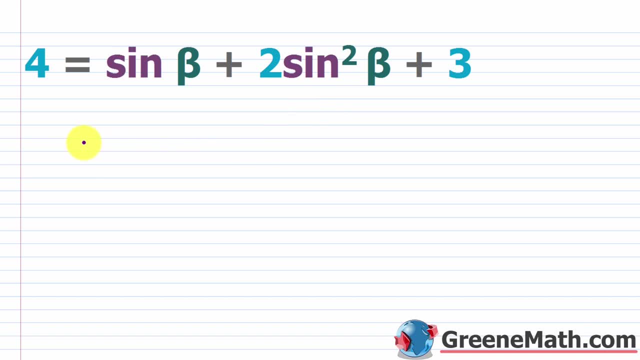 I want everything to be on the left side that I'm working with. So let's go and say we have two times sine squared beta plus let's say sine of beta. I'm going to subtract four away from each side of the equation. 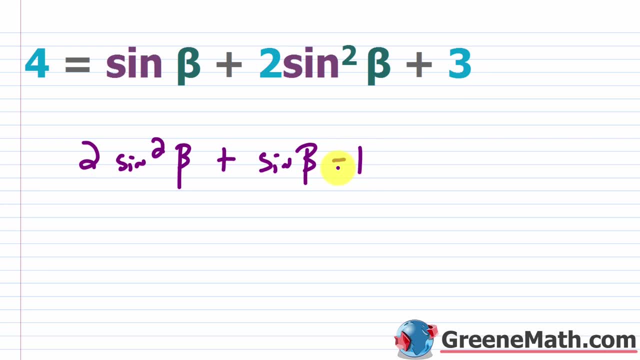 So this would end up being Basically negative one over here, because if I subtract four away from each side, this would be negative one and this equals zero. So now what I have here, I should be able to factor. So again, if you're struggling with this, if you just can't get past the mental 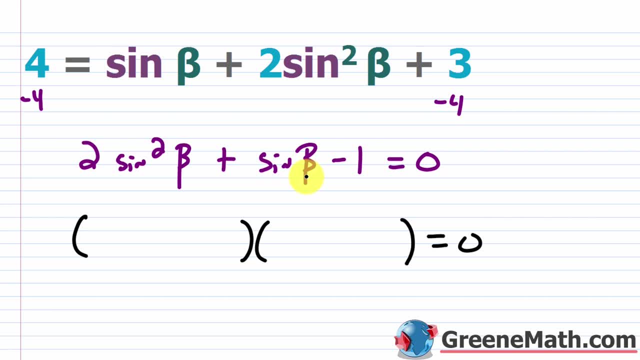 roadblock. go ahead and take sine of beta and set that equal to a variable. like you, I think we can get past it Right. So I'm just going to put sine of beta here and sine of beta here to start Now. this two in front. that's a prime number. 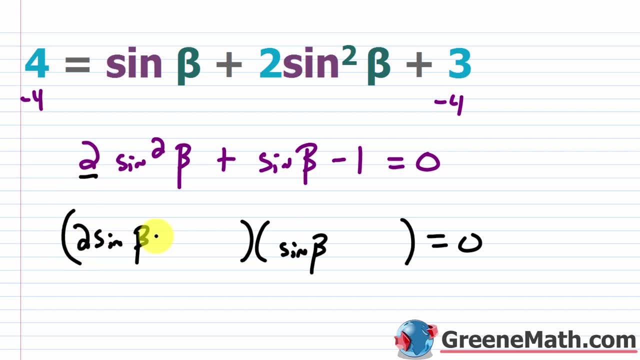 So I've got to stick that in one of these. so I'm just going to stick it here. So we have two times sine of beta, times sine of beta, which would give me two times sine squared beta. OK, so that works. Now we have alternating signs here. 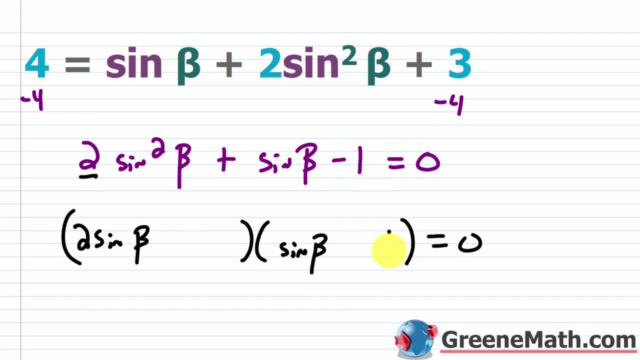 Let's think about this. We have a negative one as a final term, so it has to be one times one. But we have to think about the signs there. Is it going to be plus here and minus here, or vice versa? Well, the outer here would be two times sine of beta, but it would be negative. 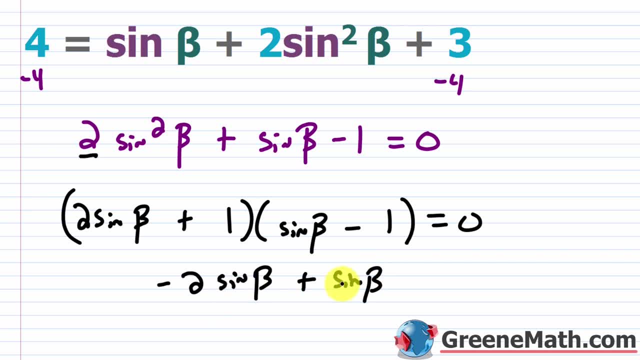 And then the inner would be plus the sine of beta. So that's not going to work, because the middle term is positive. OK, so that means I need a plus here And a minus here. So let's erase this. And now you see, it works out right. 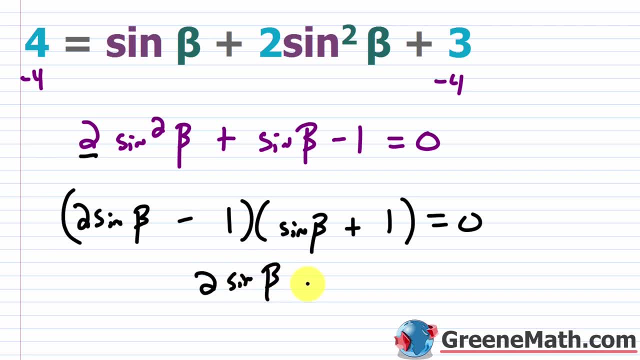 Because the outer would be two times sine of beta And then the inner will be minus sine of beta And so if I do the subtraction I get my plus sine of beta and then negative one times positive, one is negative one. So we have correctly factored this guy. 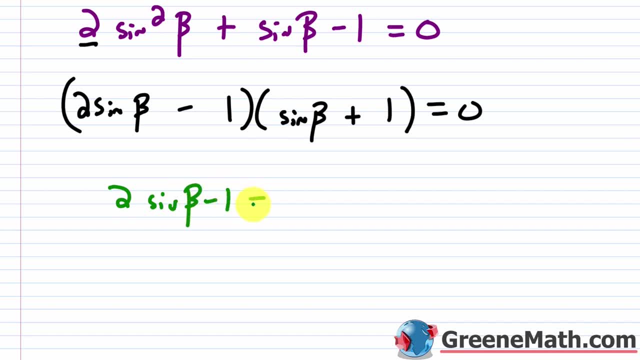 Same thing. So two times sine of beta minus one, Setting that equal to zero. Let's go and solve it. Add one to each side of the equation You get. two times sine of beta Is equal to one, And I'm going to divide each part by two here. 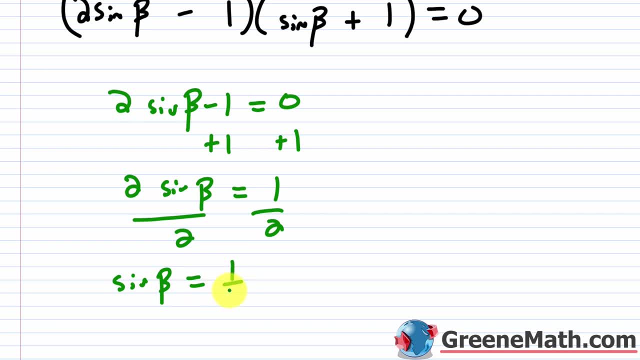 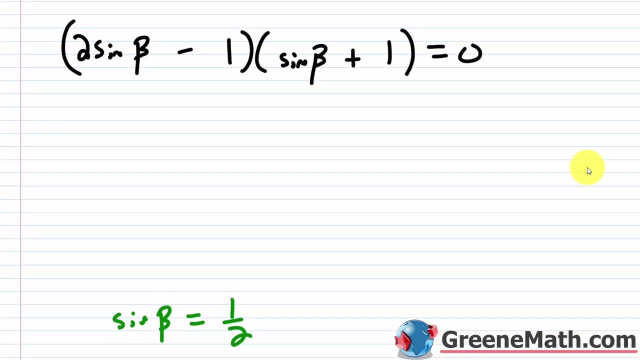 And basically I get that the sine of beta is equal to a half. So let's erase this. And you see these values so often, it's almost like you start dreaming about them. We know that this is going to be 30 degrees or 150 degrees. 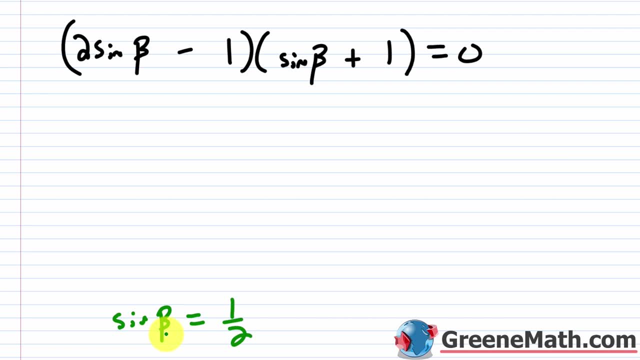 Again, if we're in that interval from zero to 360 degrees where you could say pi over six or five, pi over six in terms of rates. So let me write this over here. So sine of beta equals one One half. So right now I know beta is equal to. 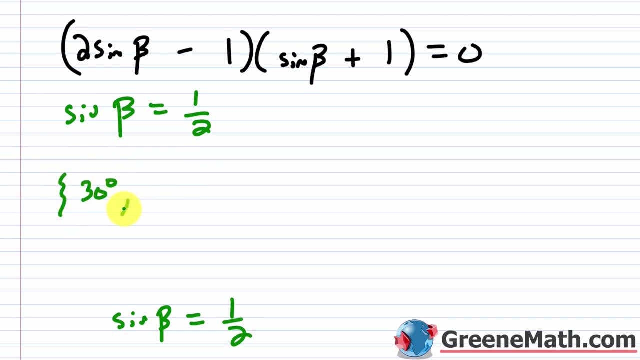 Let me just do this in solution set notation. We know we have 30 degrees and we have 150 degrees. OK, so so far that's what we got. Let me put this in terms of radiance also. So let's go pi over six and then five, pi over six. 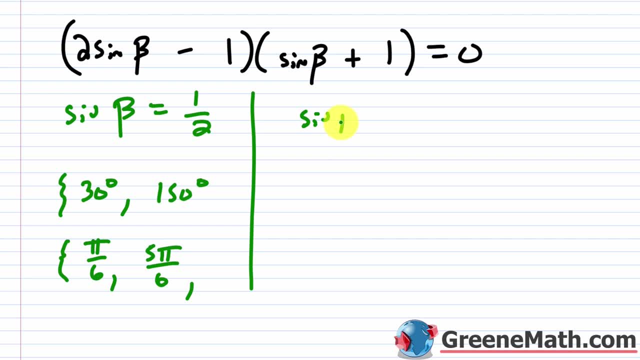 So what's going to be the result from over here? Let me draw a little line. We have the sine of beta plus one equals zero. Again, we're just going to subtract one away from each side, So the sine of beta is equal to negative one. 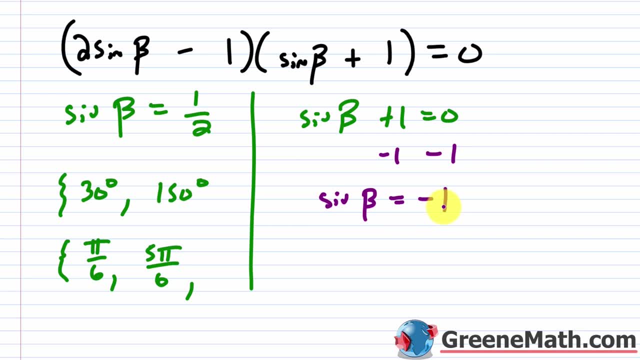 And again, if you know your unit circle, this is basically going to give us 270 degrees, or three pi over two. So let's get rid of this. Let's put 270 degrees And then, over here, let's put three pi over two. 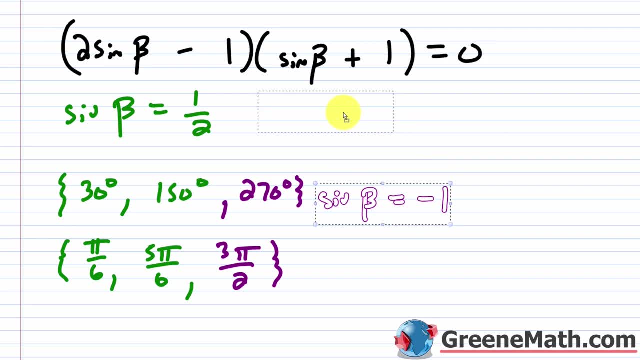 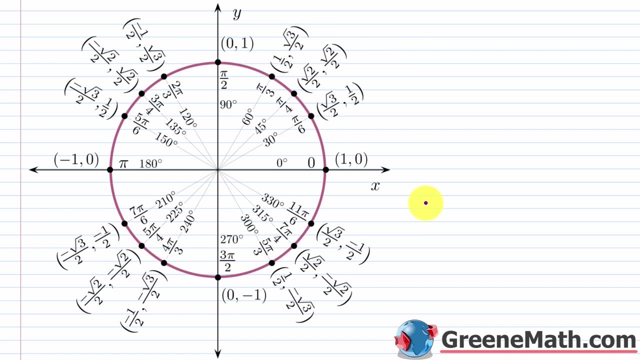 Let me just erase this real quick and let me just drag this out of the way. So we'll put this over here. So let's put or, and then let's come down here And again. the more you reference the unit circle, the more you work with it, the more you memorize it. 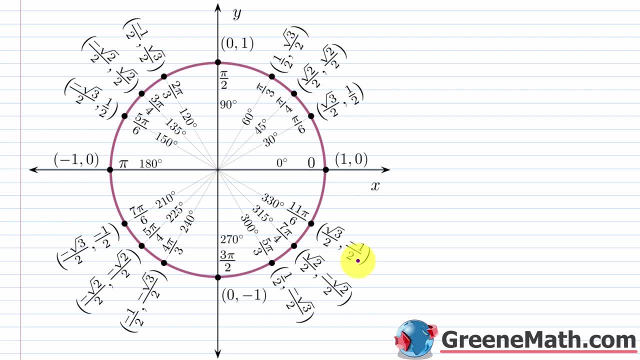 Again, we were looking for sine of beta to be equal to one half, So that's going to be here. You're looking for your Y value, So 30 degrees, or pi over six. And then, if I go in, quadrant two, where sine is positive, again, 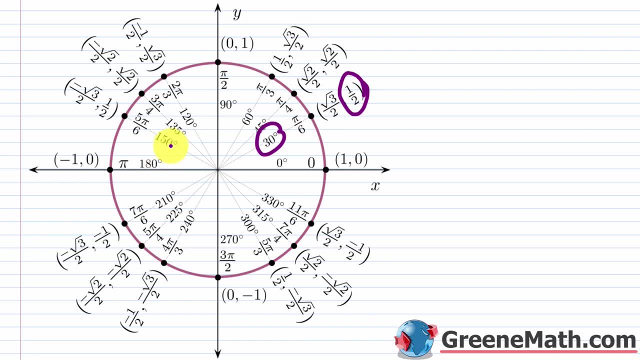 what angle is going to have? a reference angle of 30 degrees, 150 degrees, So it's going to be here. OK, it's 150 degrees, or five pi over six. Then, if you're looking for a Y value of negative one, it's going to be at 270 degrees, or here. 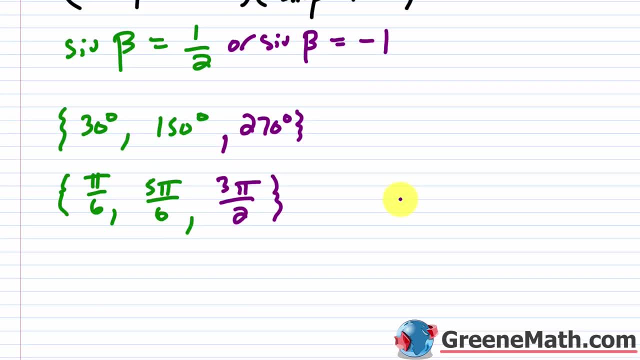 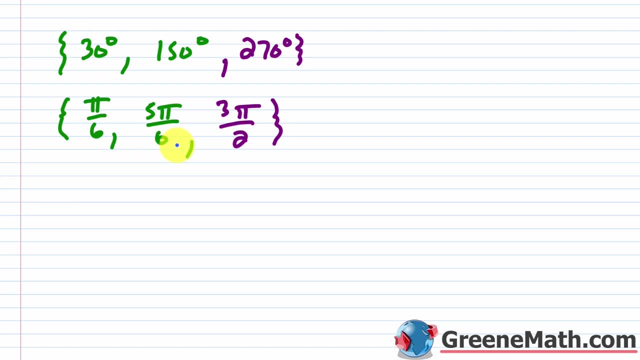 or again, three pi over two in terms of radians. OK, so let's talk about the general solution. This might not be obvious, but when you look at these, sometimes they're going to have this pattern. I know when we work with sine or cosine, they repeat every 360 degrees. 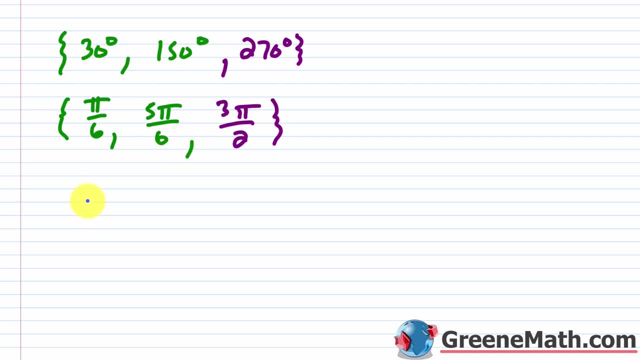 But if you notice this one, if you start it, let's say you went through and you say, OK, well, 30 degrees plus 360 degrees, 390 degrees, then 150 degrees plus 360 degrees is 510 degrees, and then 270 degrees plus 360. 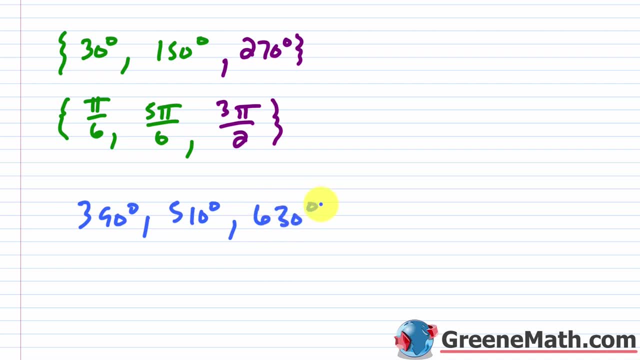 degrees is 630 degrees. So I want you to notice that everything that I have here is just differing by 120 degrees. So if I start here and go here, I added 120 degrees, I added 120 degrees, I had 120 degrees, so on and so forth. 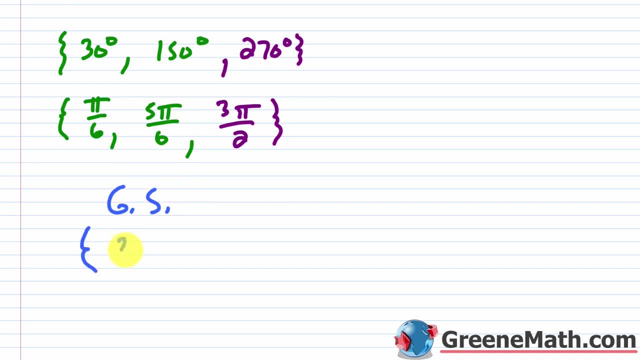 For a general solution. in this particular case I can say 30 degrees, OK, plus I know the period of sine is 360 degrees, But because of this I can say 120 degrees times that, So 30 degrees plus 120 degrees times then. this would be a simpler way to write this. 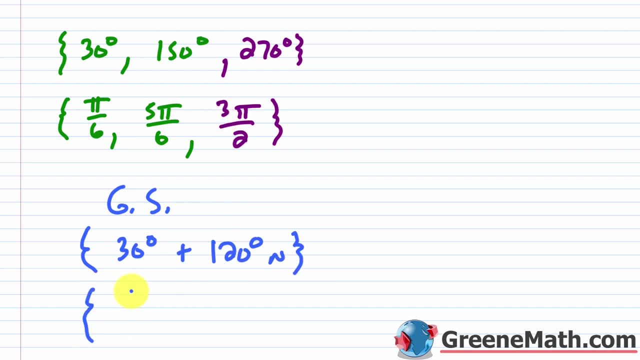 Then for this guy, if you want to put this in terms of radians, let's go ahead and just say that you have pi over six, Plus you're going to do 120 degrees in terms of radians. So that's two pi over three. 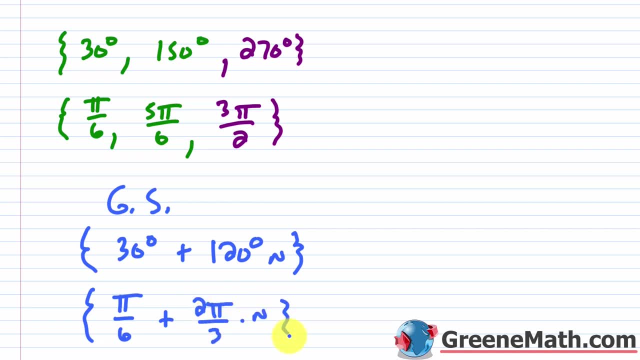 So two pi over three and then times that. OK, so let's close that up. So this would be our general solution. And then this is: if we had a domain restriction, So let's say from zero to 360 degrees, and then here let's do from zero to two pi. 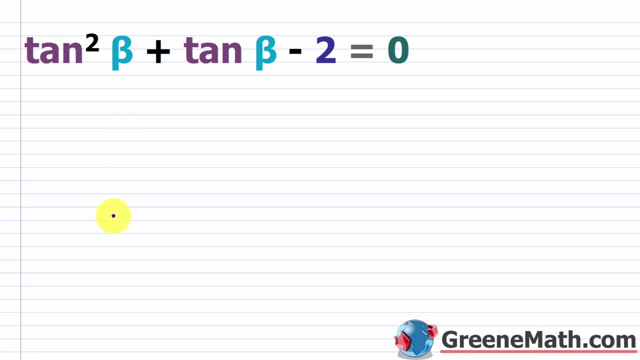 All right, let's look at one that's much more challenging. So here we're not going to be able to use our fancy unit circle. I think we can on one part, but on the other we can't. So we have tangent, squared beta plus tangent. 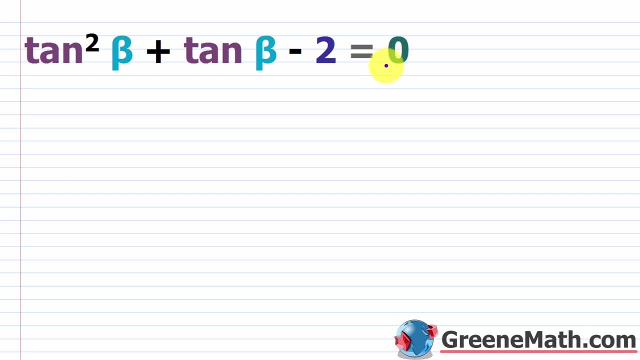 of beta minus two equals zero, So same deal. I'm going to be able to factor this and I'm just going to set this up. It's already. it's already in line for me the way I want it, So I'm just going to put the tangent of beta and the tangent of beta. 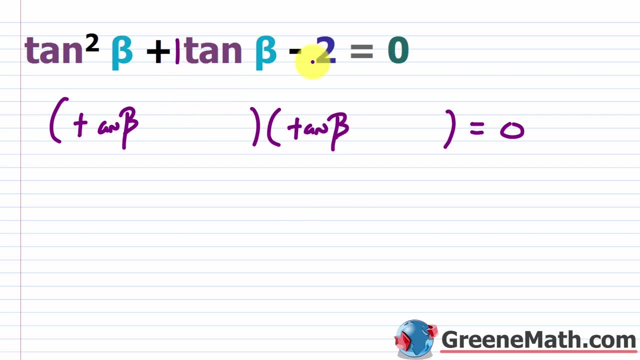 So I basically need a positive one and a negative two. So how am I going to get that? Well, basically I want to do positive two and negative one. So this guy's factored pretty easy to do that. Let's go ahead and start with the easier one. 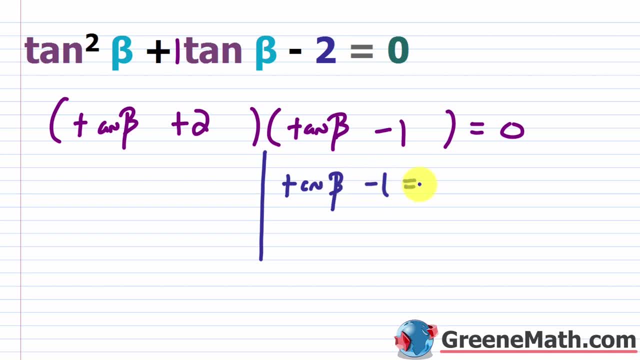 So let me start with the tangent of beta. minus one equals zero. So we'll say that tangent of beta, if I add one each side would be equal to one. So where's the tangent of beta equal to one? You might remember from your special 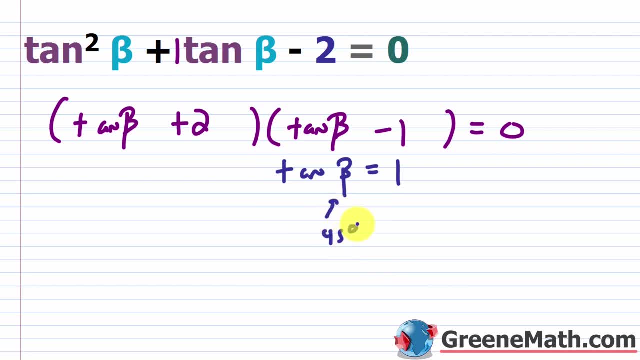 triangles, that one solution here would be forty five degrees. Remember tangent is positive in quadrants one and three. Remember the all students, the all, all students take calculus. So it's positive in quadrants one and three. OK, so I need to find the quadrant three. 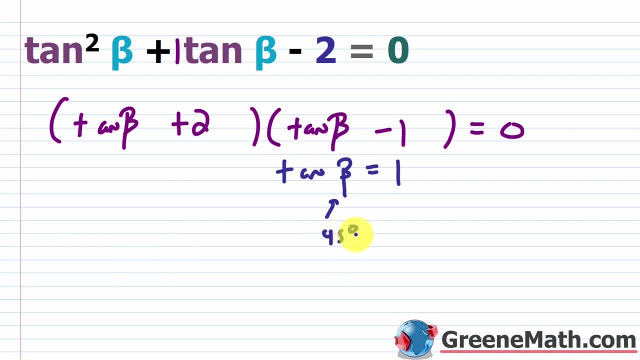 solution. So what the angle in quadrant three with a forty five degree reference angle? so I can go ahead and do one hundred eighty degrees plus forty five degrees, which is going to give me two hundred twenty five degrees. So let me put two hundred twenty five degrees to finish that up, and then I can erase it. 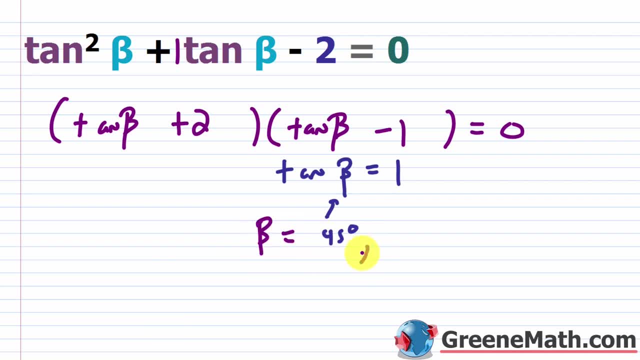 So let's put, beta is equal to forty five degrees, or two hundred twenty five degrees In terms of radians. you could write it like this: You could put pi over four and then you could do five, pi over four. So that takes care of this part. 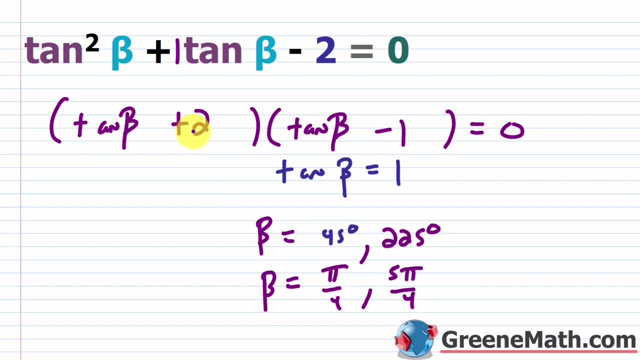 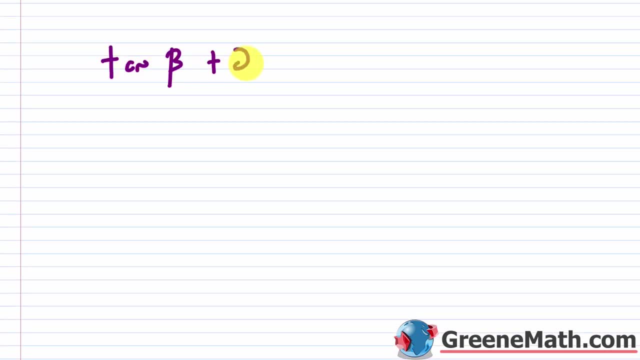 Now over here. this is where we're going to struggle a little bit. So we have the tangent of beta plus two. We're going to set that equal to zero. So let's go down here and get a lot of room, We'll come back up. So the tangent of beta plus two is equal to zero. 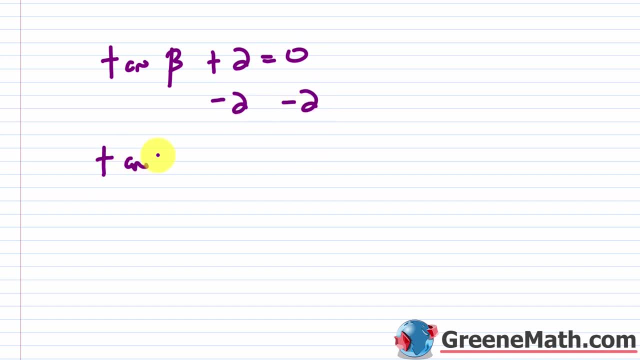 Let me subtract two away from each side of the equation I get the tangent of beta is equal to negative two, So there's nothing you can pull from special triangles or the unit circle where you're going to figure this out. OK, so what I would do here is go through and basically use. 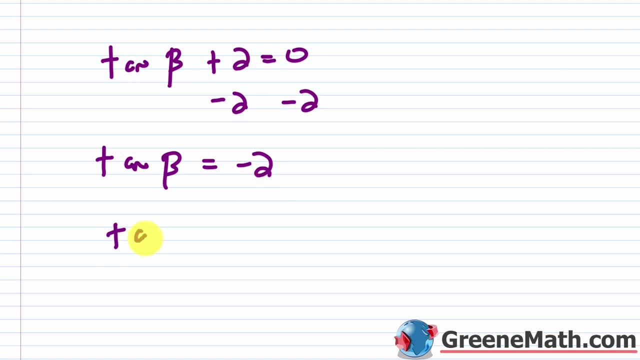 your inverse tangent function on your calculator. OK, go ahead and use this guy. OK, and I'm going to use positive two, not negative two. If you punch this up, you're going to get sixty three point, And I'm going to round this. Let's say four, three. 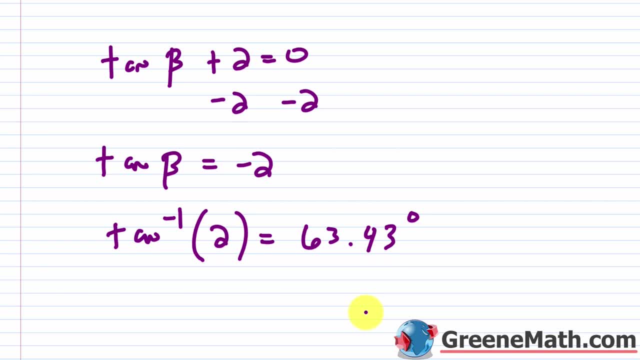 So this is in terms of degrees. So now, what this is telling me is that the reference angle with wherever I need to go is going to be sixty three point four, three degrees. Now tangent of beta here is negative. Where is tangent negative? 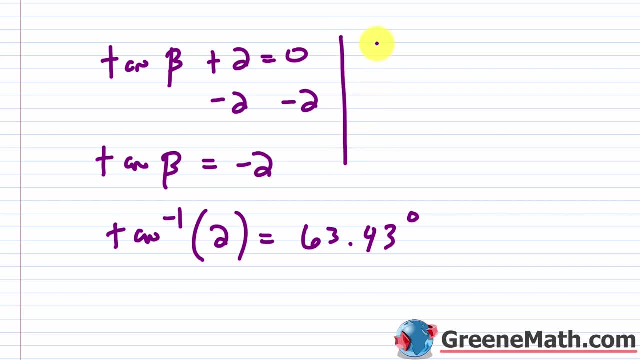 It's negative in quadrants two and four. So I'm looking for a solution in quadrants two and in quadrants four And what I want is the angle, with a reference angle of sixty three point four, three degrees. So in quadrant two I would do one hundred eighty degrees. 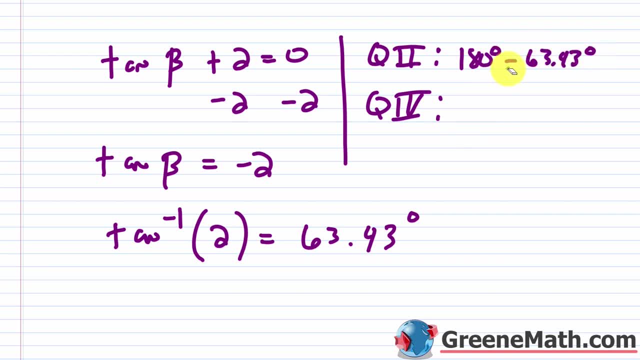 minus sixty three point four, three degrees, which I'll say is one hundred sixteen point five, seven. So let's go ahead and write this as one hundred sixteen point five, seven degrees, And then in quadrant four I would do three hundred sixty degrees minus this. 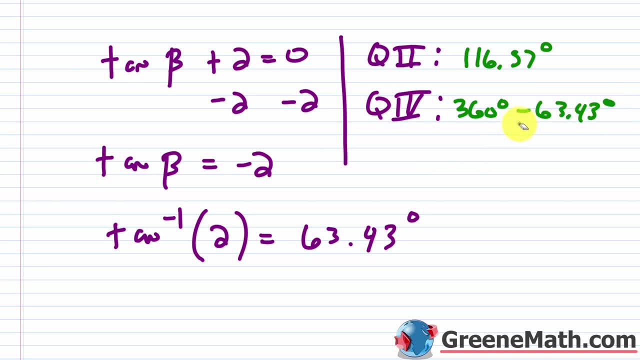 sixty three point four, three degrees, And that would give me two hundred ninety six. Let me write this down: So two hundred ninety six point five, seven degrees. So let's erase all of this. We don't need it anymore And let's just bring this up here. 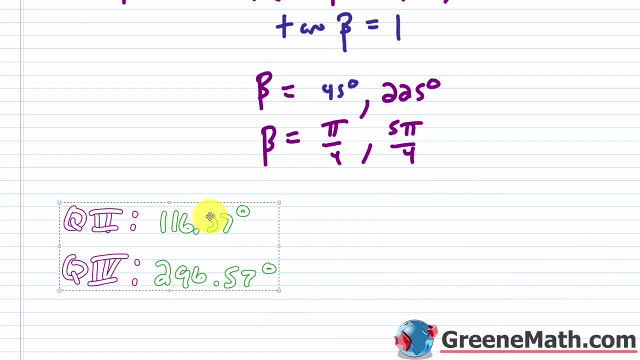 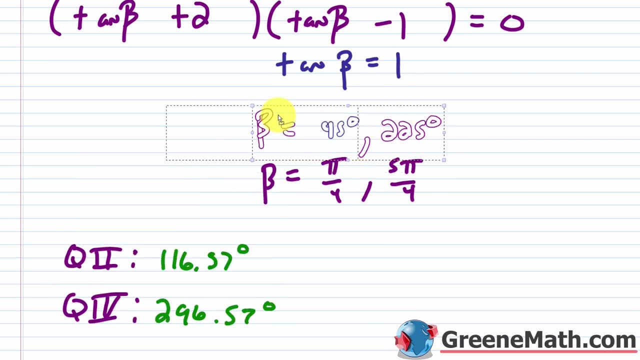 And I'm going to combine all of this for one solution. Let me get this over here and let me come up here And I'm basically going to say, and let me kind of drag this over here. So I'm going to do one four degrees and one four. 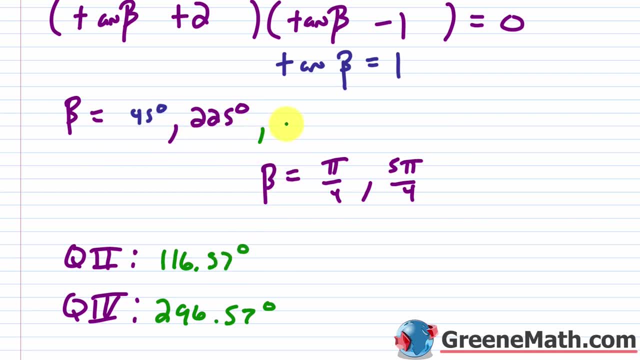 So beta could be forty five degrees, two hundred twenty five degrees, You could have one hundred sixteen point five, seven degrees, And this is an approximation. So maybe you want to notate that this is approximately here, And then this is an approximation also. 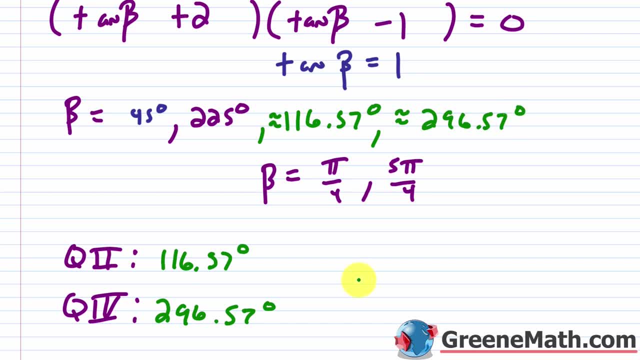 So two hundred ninety six point five, seven degrees, And then in terms of radians. if you wanted to convert this over again, for each of these you would multiply by. you have degrees here, So you want degrees down here, and then you want pi up here. 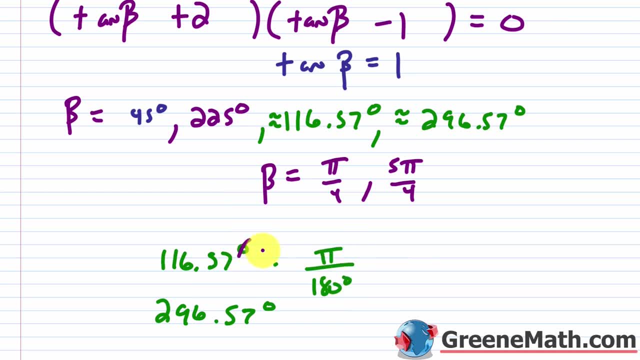 So you would basically say that the degrees are going to cancel. So let me just show that real quick: One hundred sixteen point five, seven, divided by one hundred eighty, and then I'm just going to multiply it by pi And I'm just going to round this off and say it's about two point zero three four. 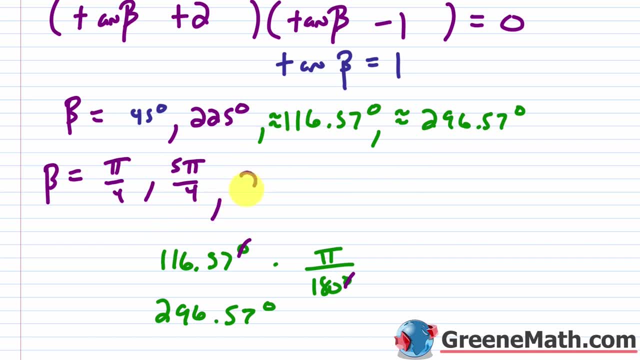 So let me slide this down and I'll just say it's about two point zero, three, four. So let's get rid of this one and let's do this one. So let's move this up And basically we're going to multiply by again. 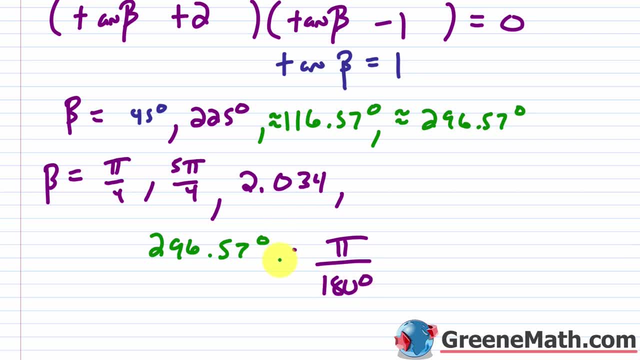 You want pi over one hundred eighty degrees. We know that the degrees here are going to cancel And basically I'm doing the same thing on my calculator: Two hundred ninety six point five seven, divided by one hundred eighty times pi. So let's just go ahead. 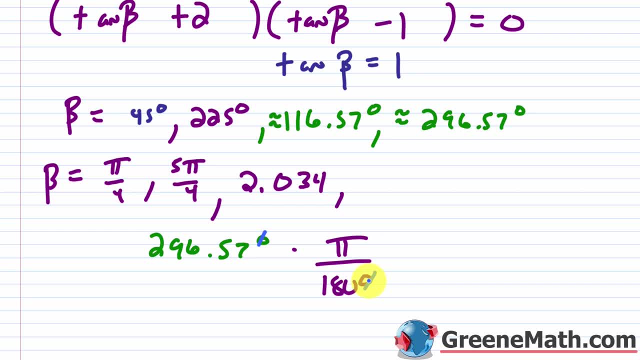 And say this is going to be five point one, seven, six. So five point one, seven, six. And again you just want to show some way like hey, this is an approximation. So I'll just put approximately like this, just showing that this is not an exact value. 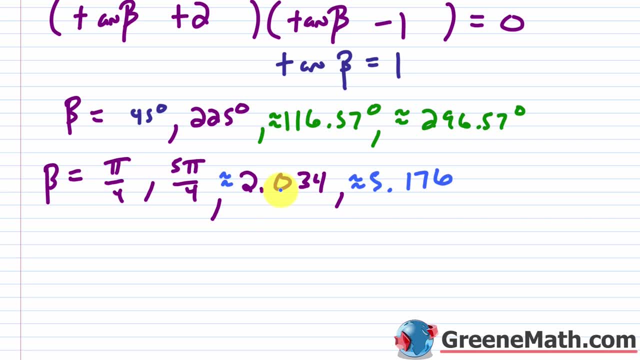 Now remember, if you're working with tangent, the period is one hundred eighty degrees, or it's pi radians. OK, so this would be for in the case of from zero to three hundred sixty in terms of degrees, And I made that terribly OK. so three hundred sixty. 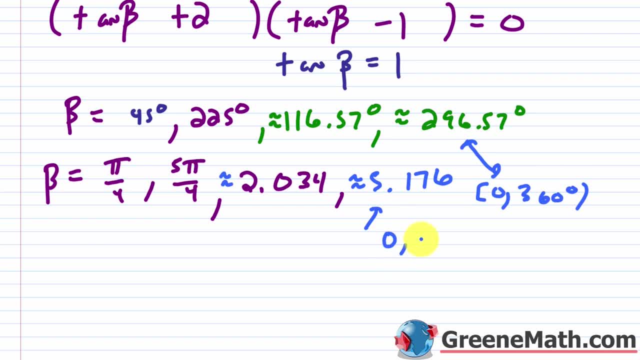 degrees, And then this would be basically from zero. Let me put my degree symbol there: Zero to two pi. And then for the general solution, I'm going to take forty five degrees. Let's go and say forty five degrees plus, I'm going to do one hundred eighty. 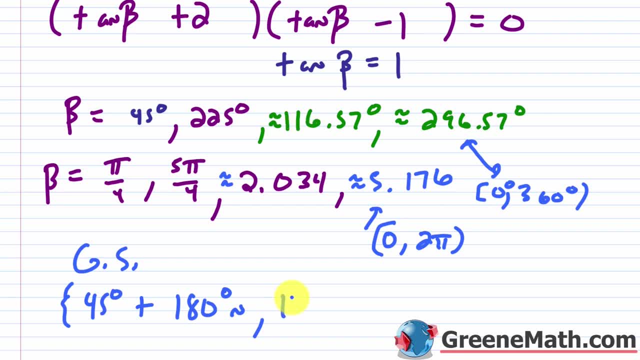 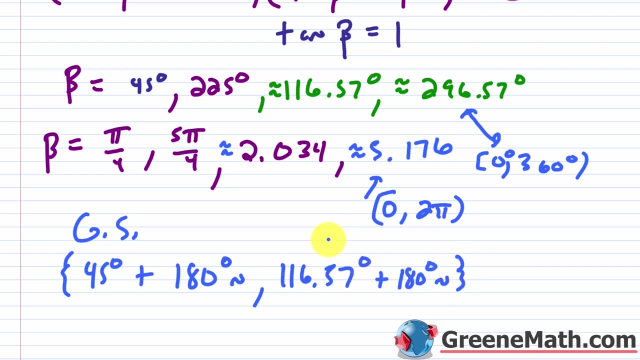 degrees times n, and then I have another guy here, So I'm going to do one hundred sixteen point five, seven degrees plus one hundred eighty degrees times that. So again, this is an approximation. This is an approximation. It is not an exact value. 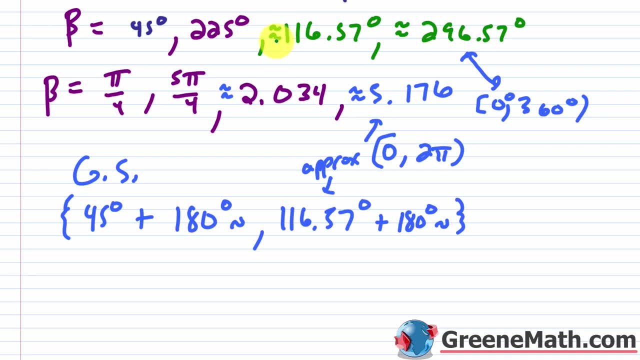 Depending on your teacher, you might have to show that in some way, So that's why I put this here and this here and this here and this here. That's just my way of notating. This isn't standard. This is my way of notating that. hey, this is an approximation. 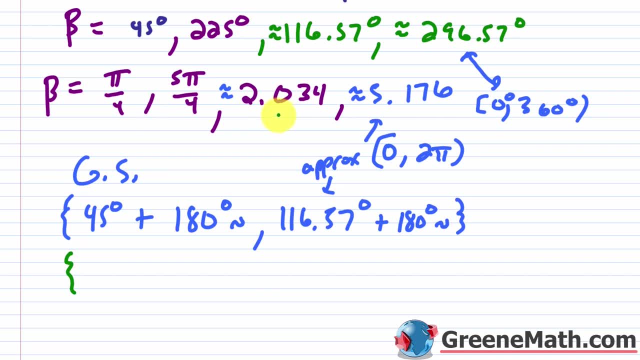 It's not an exact value. So then down here for this guy I would start with pi over four and then plus the pi times n, and then for this one I would take my two point zero, three, four and then plus my pi n. OK, like this: 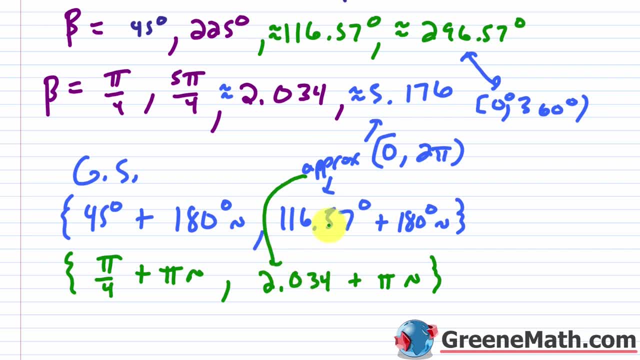 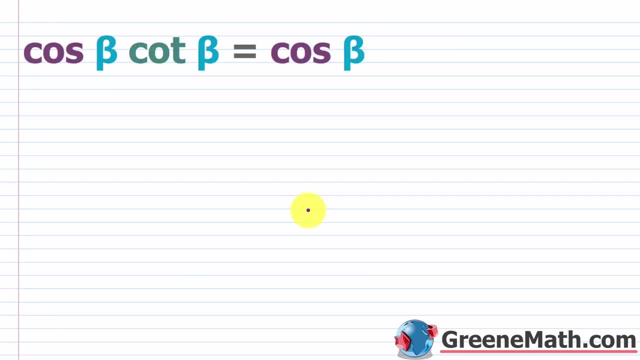 Now again, if you want to just notate that this is an approximation, and this is an approximation just to let your teacher fully know that you're aware that this is an approximation and not an exact value, All right, Let's take a look at one more problem. 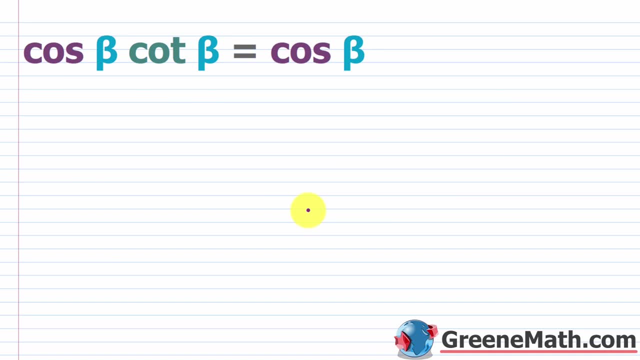 So somewhere in your textbook they're going to tell you that you don't want to divide both sides of an equation by a trigonometric function such as the cosine of beta. So when you do this, you could potentially remove some of your solutions. 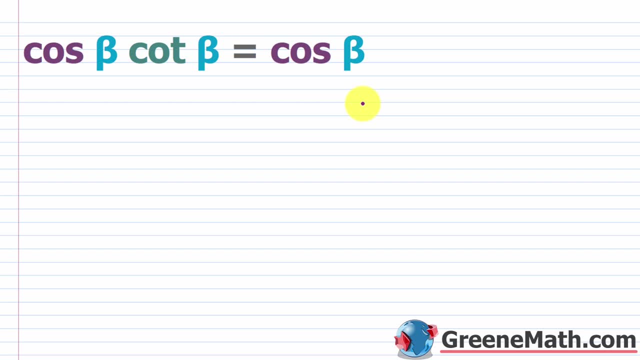 These are going to be solutions that make the divisor zero, So what I'm going to do is solve this in two different ways, and I'll show you how this can cause problems. So the first way is the correct way, and that's with factoring. 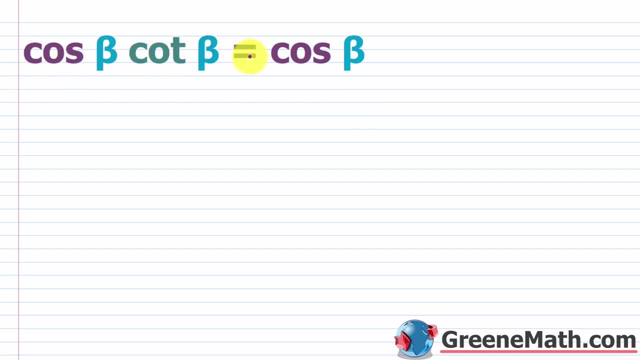 So if you have the cosine of beta times the cotangent of beta and this equals the cosine of beta, you could subtract the cosine of beta away from each side of the equation. So over here this would cancel and you'll have zero. So on the left you would have the cosine of beta then times the cotangent of beta. 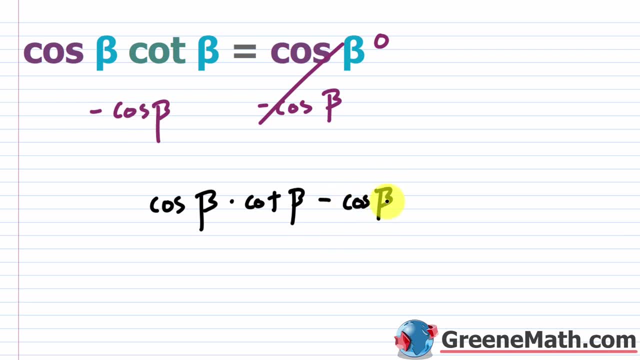 And then minus this cosine of beta And what I'm going to do, because we're going to factor this out. let me put times one, so nobody gets lost, and I'm going to set this equal to zero. Let me actually get rid of this, because 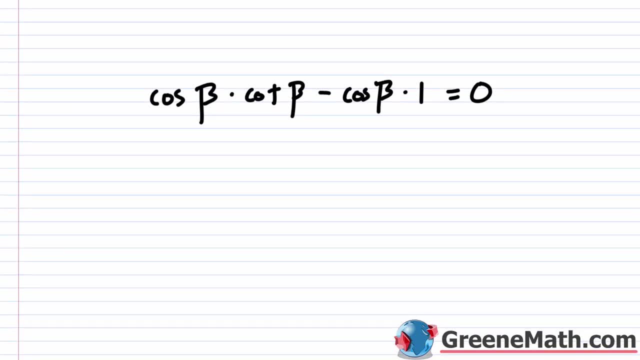 we're going to come back up and use that in a moment. So let me slide down here just a little bit and I'm just going to factor out the cosine of beta. So this right here is going to get pulled out in front of some. 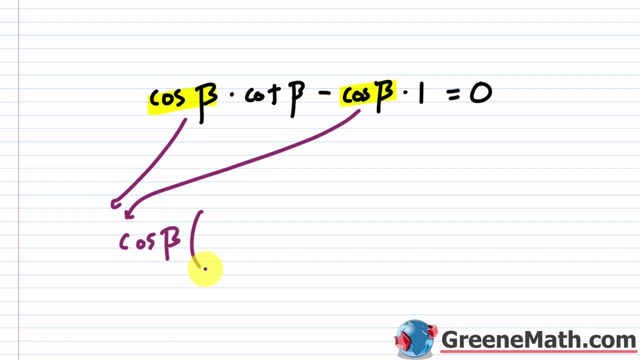 parentheses. So you have the cosine of beta times the quantity. Inside. you would have the cotangent of beta And then minus. if you pull this out, you would have your one and then close that down, and this equals zero. So we're now going to solve this using 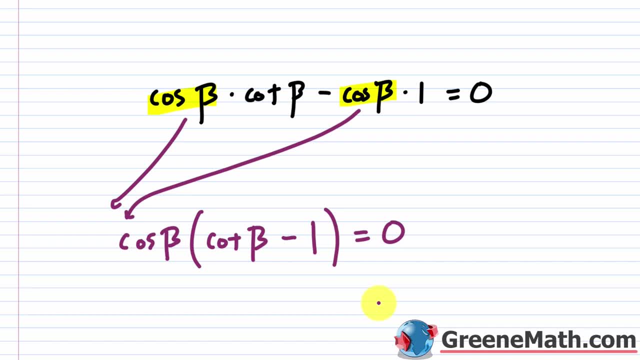 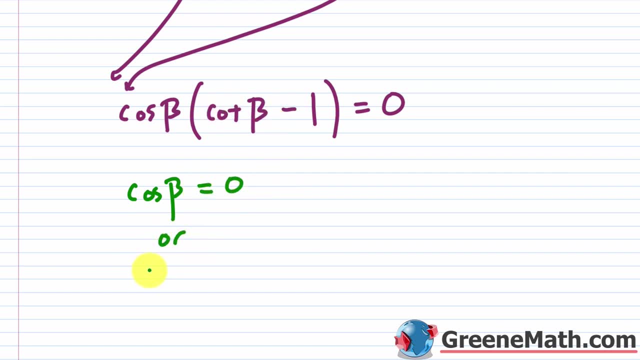 the zero product property, or you can call it the zero factor property. So for that I'm going to take the cosine of beta and set that equal to zero. Then I'll say: or I'm going to take this other factor, so the cotangent of beta minus one, and set that equal to zero. 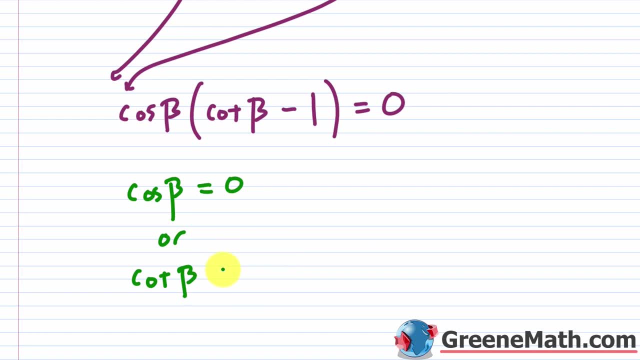 Well, for this one you can add one to both sides, So the cotangent of beta would be equal to one, And we know that the tangent of beta is equal to one over the cotangent of beta. So the tangent of beta here would be one over one, which is one. 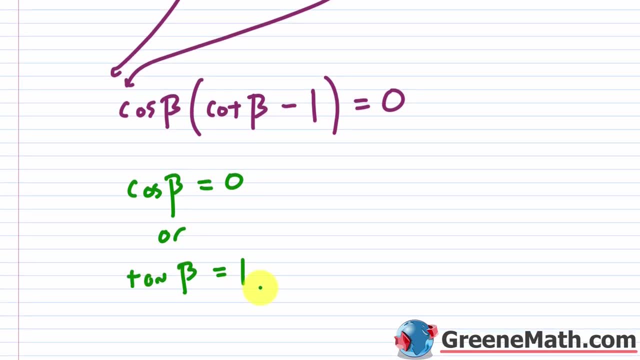 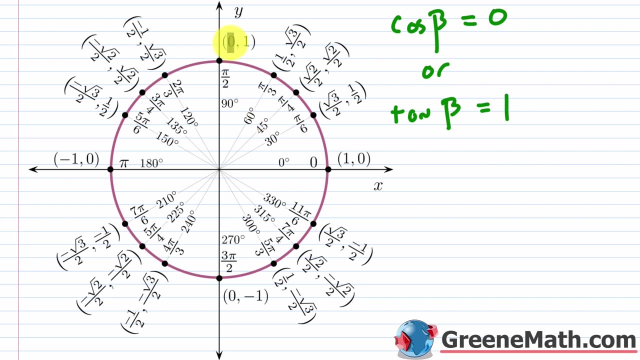 So let me write this as the tangent of beta equals one. So the first one is the cosine of beta equals zero. So I'm looking on the unit circle for an X coordinate of zero. So that's going to occur right there at pi over two or 90 degrees, and then right there at three pi over two or 270 degrees. 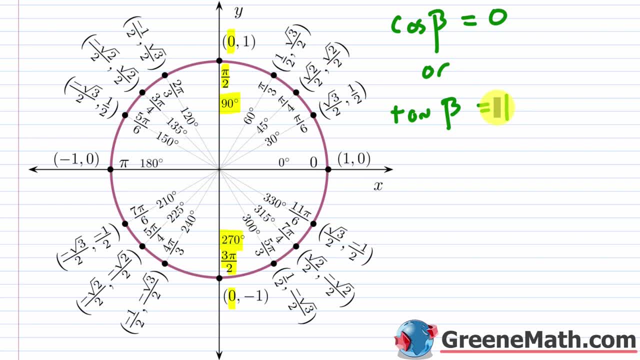 Now for the tangent of beta equals one. we've seen this several times already. We know that in the first quadrant this is going to be pi over four. Again, if you skip the other problems, you could just do the inverse tangent function with one as the argument. 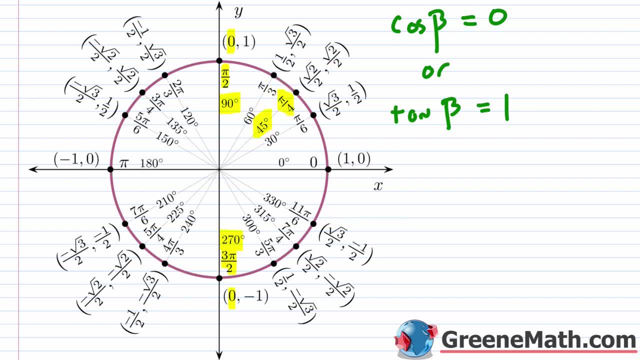 You'll get pi over four or 45 degrees. You could also think about this with the definition of tangent. So you could say that the tangent of beta is equal to the sine of beta over the cosine of beta And in this case, if you replace beta with that angle, 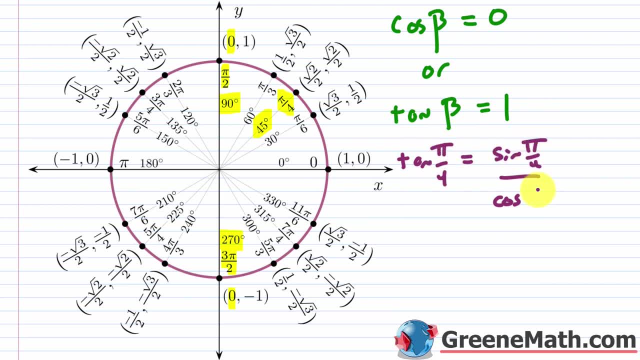 which is pi over four. you can go to the unit circle and actually see why we're getting the value of one, And that's because we have the same nonzero number divided by itself. The sine value is square root of two over two. The cosine value is square root of two over two. 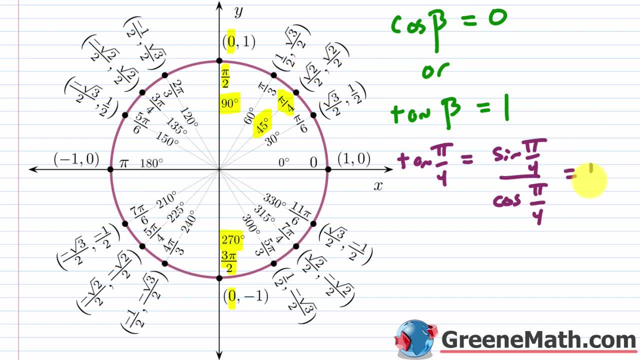 So square root of two over two, divided by square root of two over two, will give you one. And then the period for tangent is pi. So if I add pi radians or 180 degrees, that's going to give me my solution. that's in quadrant three. 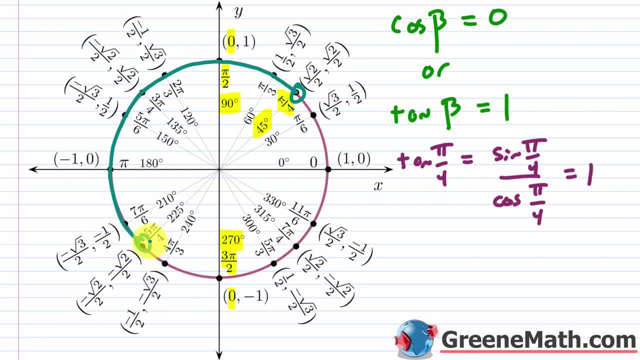 So that's going to be at five pi over four and the tangent of five pi over four, Again, you would have the same nonzero number divided by itself, And so you would get one. So let me get rid of this And let me highlight this over here as five pi over four or 225 degrees. 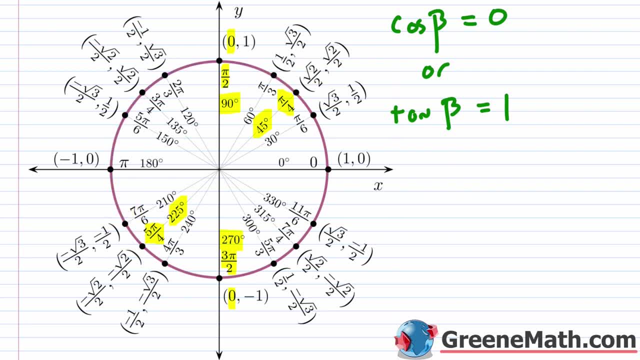 And I'll get rid of this and this and this. So if you wanted to write out your solution, you could say that beta is equal to: let's start with pi over four, and then let's go to pi over two, and then let's go to five pi over four and let's go to three pi over two. 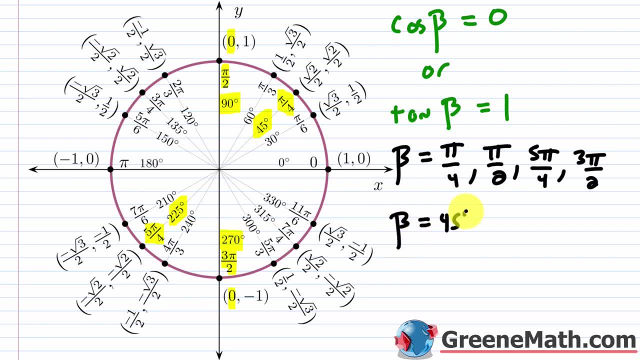 If you want to work with degrees, we could say that this is 45 degrees, this is 90 degrees, this is 225 degrees And then, lastly, 270 degrees. OK, let me grab this real quick and let me come back up here and paste this in here. 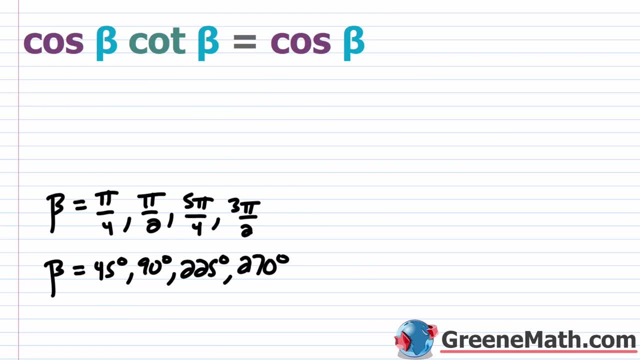 And I'm just going to show you real quick that these solutions all work, just so that when we get to the next part, you're not lost in terms of whether we did it correctly or not. So the first solution was pi over four, So let's plug that in there and there and there. 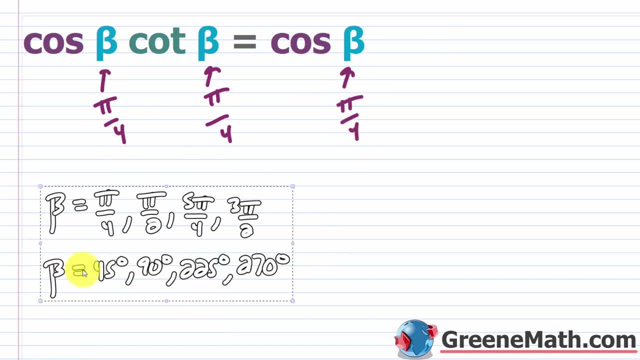 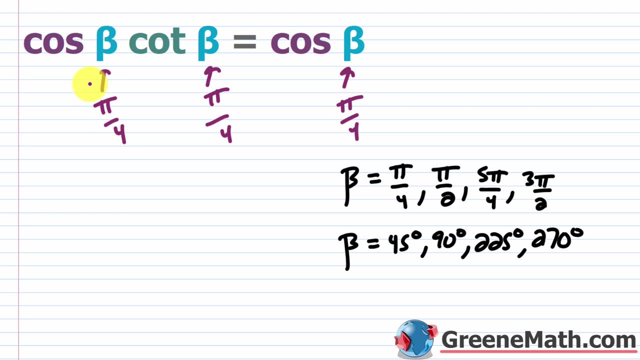 And let me make that a little bit better there. Let me slide this out of the way so we can fit this: We know that the cotangent of pi over four is one and the cosine of pi over four is square root of two over two. 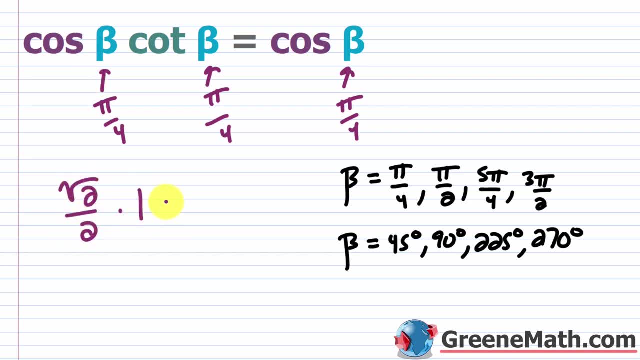 So this would be: the square root of two over two times one is equal to the square root of two over two, So that is a valid solution. Now, similarly, if you do five pi over four, the only thing that's going to change is the cosine of five pi over four. 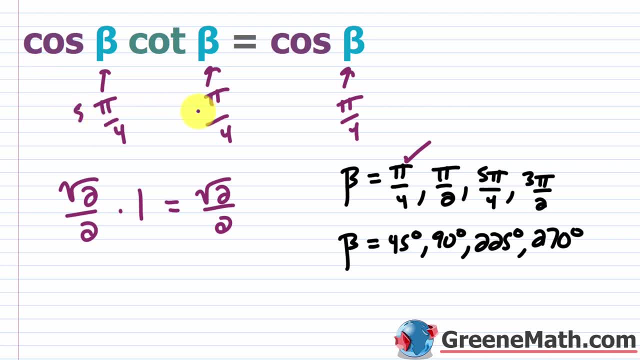 That's going to be a negative square root of two over two. So if I did five pi over four, five pi over four and five pi over four, this would be negative square root of two over two times one equals negative square root of two over two. 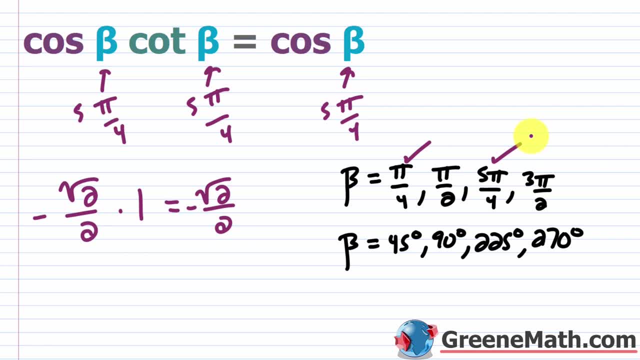 So that one's going to work as well, because you get. the negative of the square root of two over two equals the negative of the square root of two over two. Now the other ones are going to make the cosine of beta equal to zero. 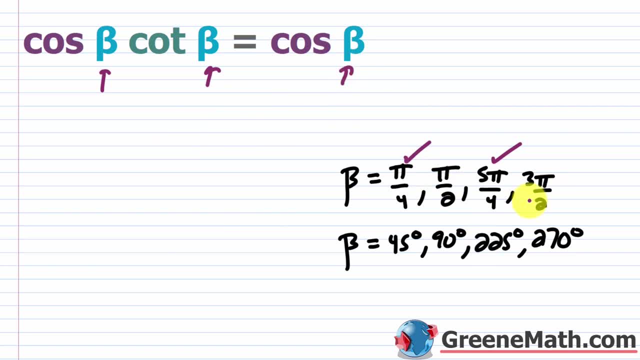 So whether you did pi over two or three pi over two, when you plug that in, let me just do pi over two- you're going to get zero equals zero, And let me make that a little bit better. there, Cosine of pi over two is zero. 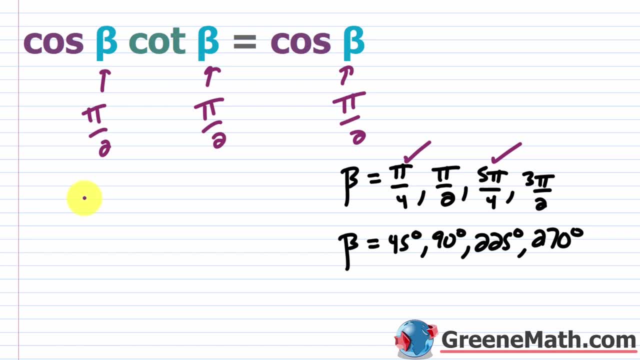 Cotangent of pi over two is actually also zero. So you would get: zero is equal to over here. Cosine of pi over two is zero, So this one would work, And so with this one it's the same thing. So you can see these solutions work in our interval. 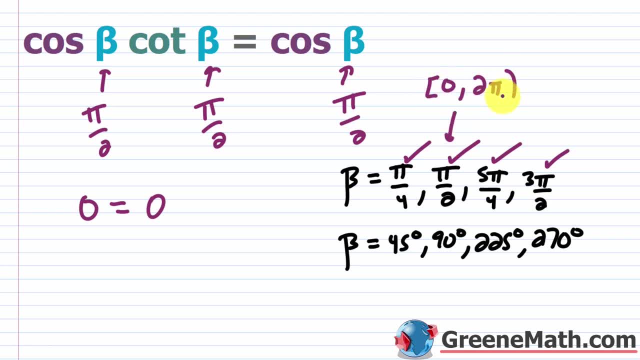 So from zero and including zero, going out to two pi- two pi is excluded. And then for this one you would have: from zero degrees, where that's included, going out to 360 degrees, where that's excluded. OK, let me get rid of this. 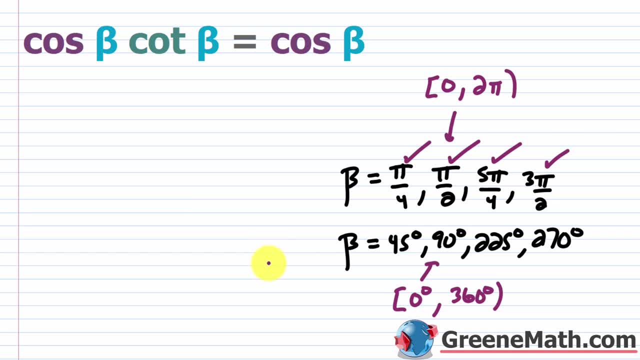 And let me show you what can happen If you solve this in a different way. So let's say, instead of factoring, I decided I was going to divide both sides of the equation by the cosine of beta. So let's divide this side by cosine of beta. 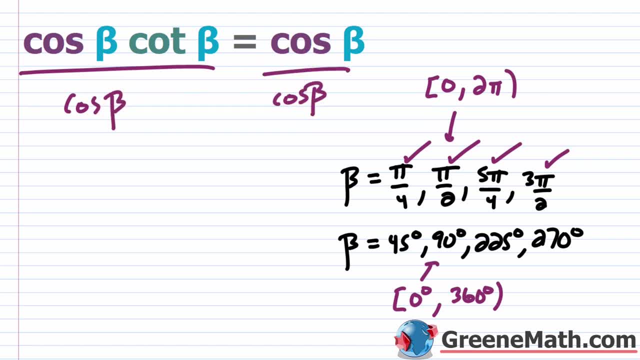 And let's divide this side by cosine of beta And you're going to see a problem happen. So this would cancel with this And you'd have the cotangent of beta is equal to. Well, this would cancel with this And I have a one, So it equals one. 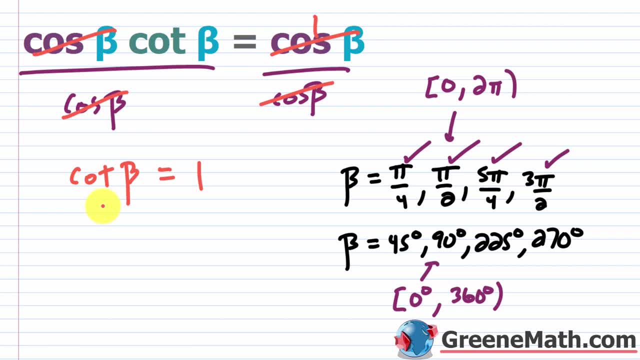 OK, well, we know this turns into the tangent of beta equals one And we know we get this solution right here, So pi over four, and we get this solution right here, which is five pi over four. But what happened to these solutions right here of pi over two and three pi over two? 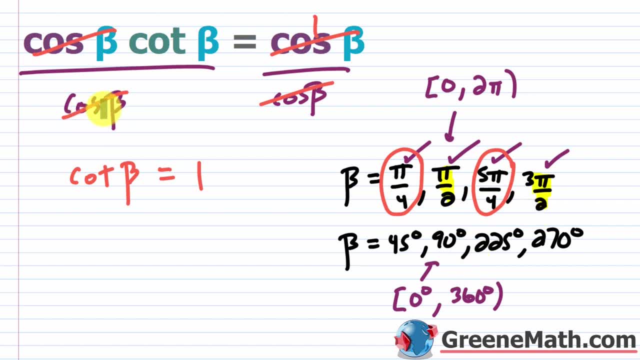 Well, those are the solutions that make this divisor zero. Cosine of pi over two is zero. Cosine of three pi over two is zero. So that's what's going on. You're going to potentially remove solutions if you use this strategy. 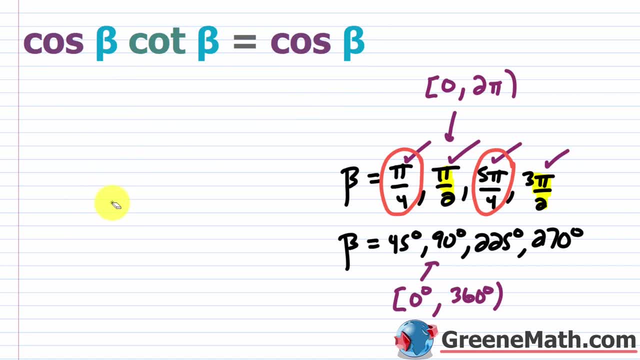 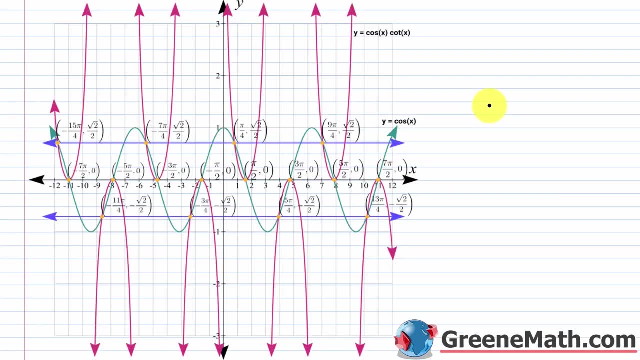 So what we want to do is stick to factoring when we try to solve this type of problem, because you're not going to run into these types of issues. So I just want to note real quick for those of you that are interested: 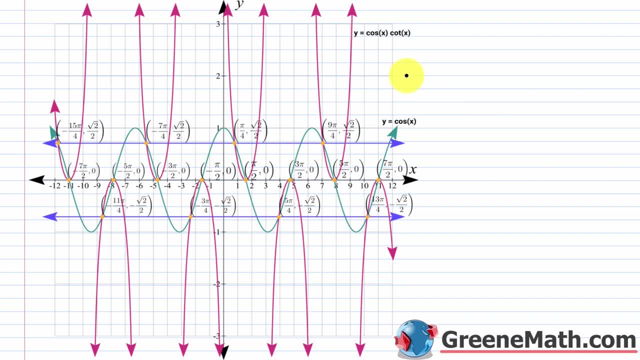 you can look at this problem on Desmos. What you would want to do is go back to the fact that you have the cosine of beta. I'm just going to call it the cosine of X times. The cotangent of X is equal to the cosine of X. 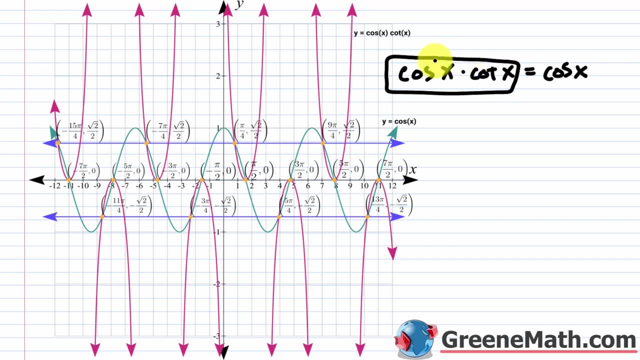 Now what you're going to end up doing is graphing this guy on the left and this guy on the right separately. So the graph in red is Y equals the cosine of X times the cotangent of X. in the graph in green is Y, equals the cosine. 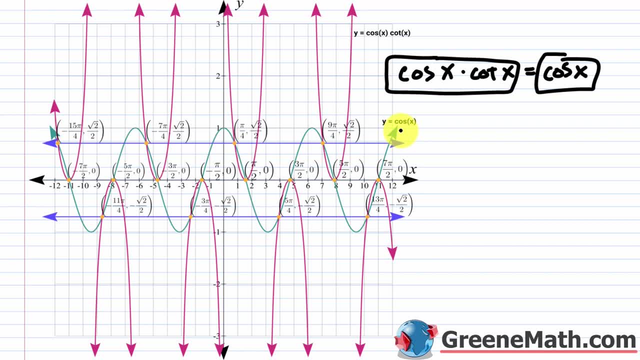 of X. So if you want to solve it this way, you're looking for the points of intersection between those two graphs. So you're basically asking the question: for which X values are the Y values going to be the same? those are going to satisfy the equation. 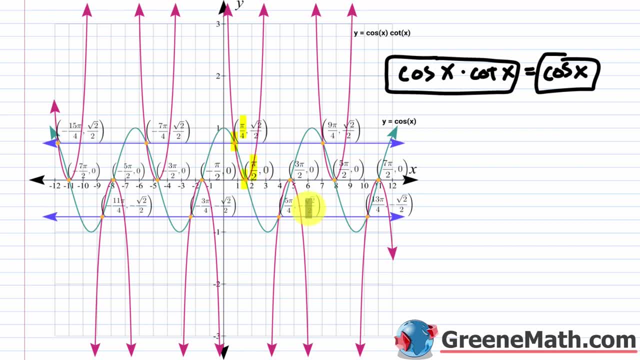 So the ones we found, we found pi over four, We found pi over two, We found five pi over four And then we found three pi over two. So you can continue with that if you want. This is something you can look at on Desmos on your own. 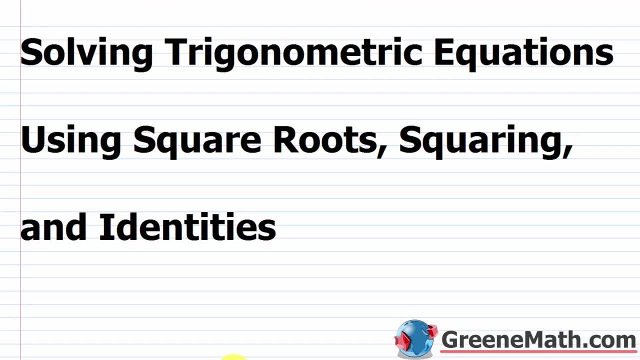 If you want a visual representation of what's going on In this lesson. we want to talk about solving trigonometric equations using square roots, squaring and identities. All right, So let's go ahead and start off with four times sine squared: beta minus one equals zero. 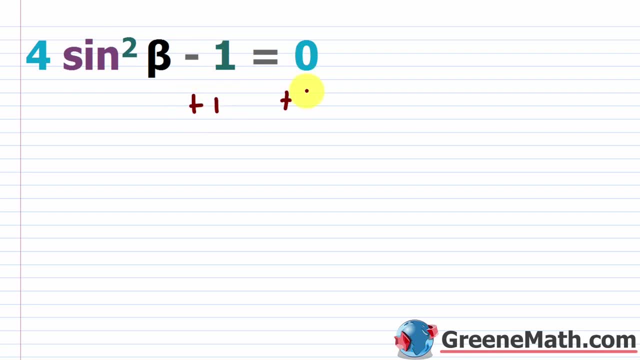 So, just like we've been doing before, we're going to add one to both sides of the equation. We're going to have four times sine. squared beta is equal to one. Okay, So what I want to do now? remember, you're always trying to isolate your trigonometric expression. 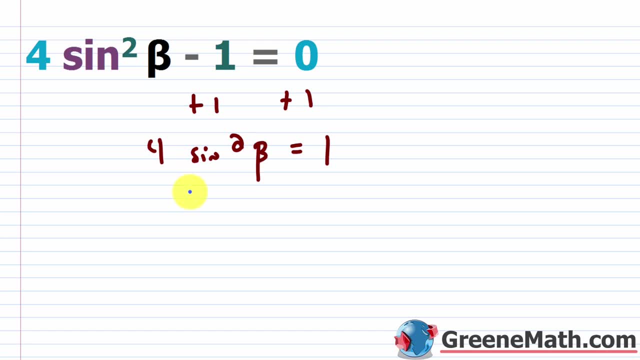 So I want sine of four. I want sine of beta by itself. So what I'm going to do here is just divide both sides by four, Okay, And so that's going to give me the sine: squared beta is equal to one fourth. 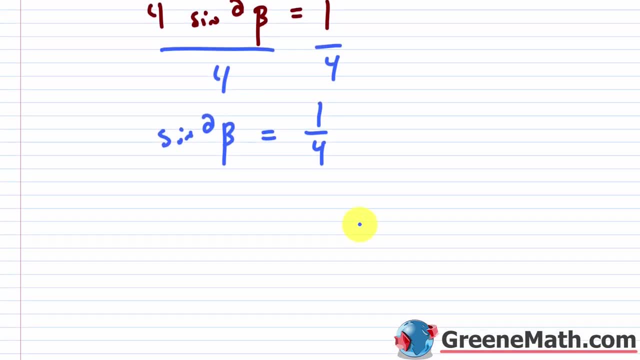 Okay, Let me scroll down just a little bit and get some room. So now, because this guy is squared, I want to take the square root of each side. Remember how this works If I take the square root of the left. on the right, I want to go plus or minus. 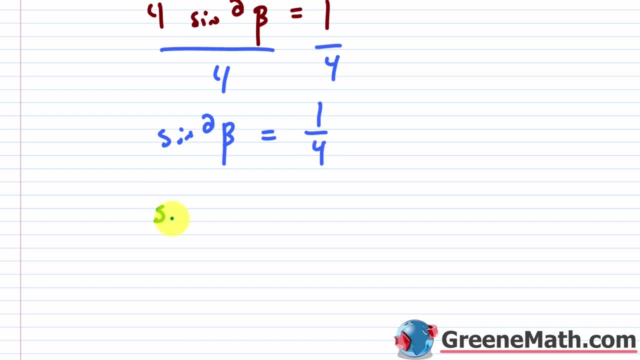 Right To account for the positive or the negative. So I'm going to say that the sine of beta is equal to plus or minus, The square root of one. fourth. Okay, If you simplify this, you'll say the sine of beta is equal to, you'll go plus. 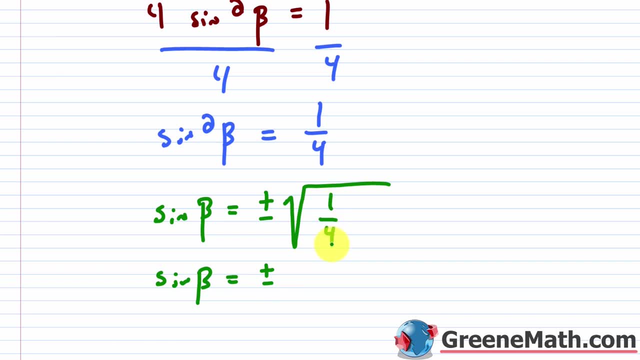 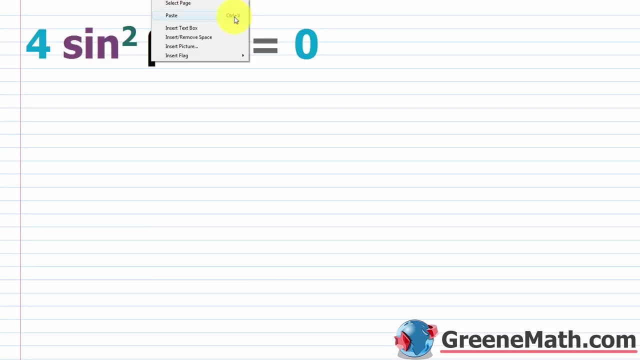 or minus. the square root of one is one in the square root of four is two, So you can basically say this is one half Okay. So let me actually erase all of this And let's come up to the top and just paste this back in here. 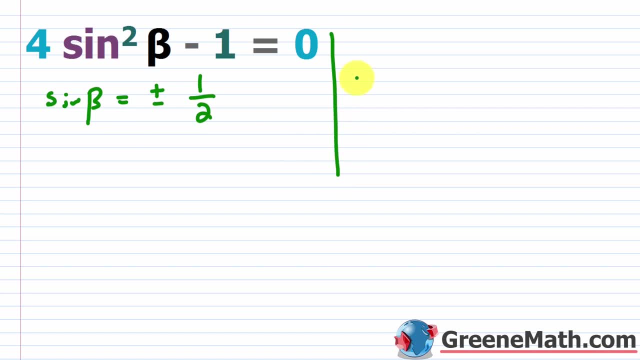 So we know this gives us two scenarios, Right? So I want to split this up and say: the sine of beta is equal to one half, or the sine of beta is equal to the negative of one half. So let me erase this now. Okay, So we have our two guys there. 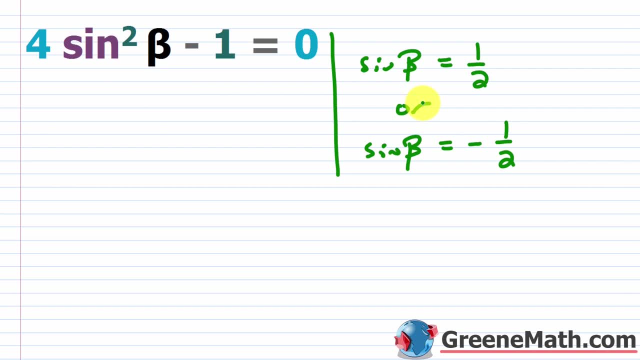 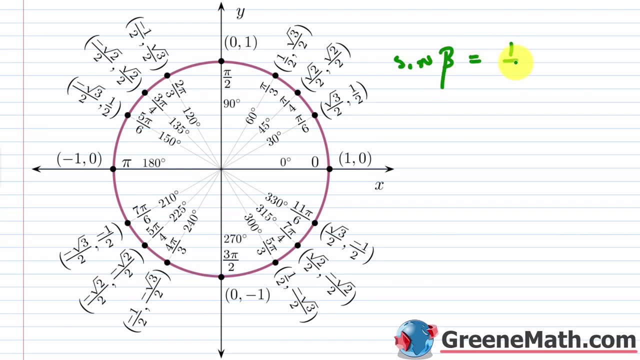 So basically, what I'd want to do is go to my unit circle. I know at this point a lot of you already have it memorized, but some don't. So let's go down and let's look for where the sine of beta is equal to a half, and then also where the sine of beta is equal. 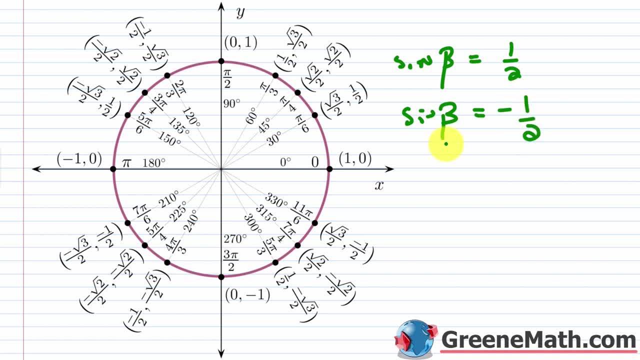 to negative one half. So basically, you're looking for your y coordinate to be a half or negative one half. So that's going to happen here. Okay, It's also going to happen as we go around. It's going to happen here as we go around. 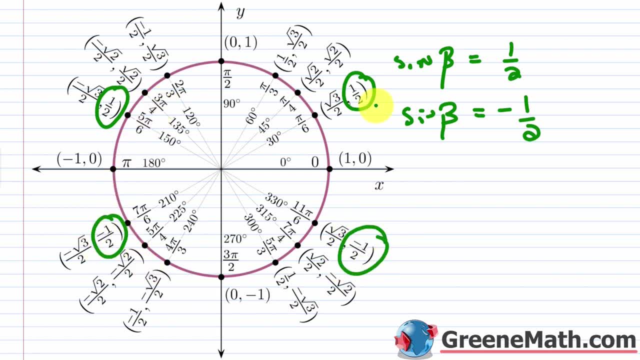 It's going to happen here And then, as we go around, it's also going to happen here, Okay, So notice, everywhere where I circled has a 30 degree reference angle, Right. So basically it's going to be, if you want. 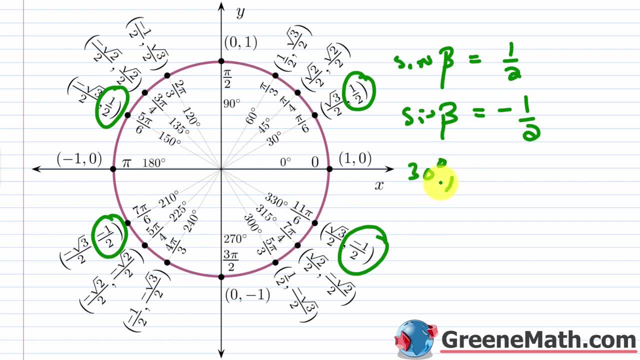 to put this in terms of radians or degrees. we'll just do both. So 30 degrees, then you have 150 degrees, You also have your 210 degrees and then you have your 330 degrees. Okay, So that's in terms of degrees. 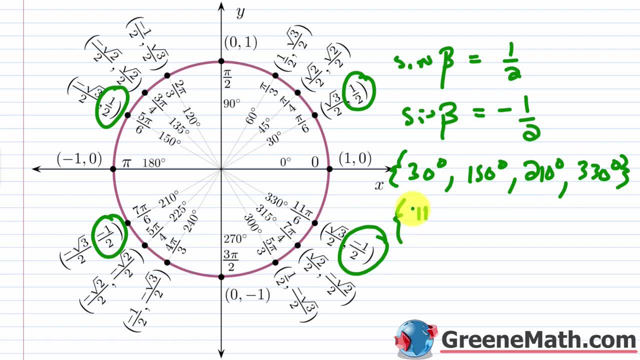 And then, in terms of radians, you would have your pi over six. Okay, You would have your five pi over six, You would have your seven pi over six And then, lastly, you would have your 11 pi over six. So these would be your solutions. if you said between zero and 360 degrees, or also, 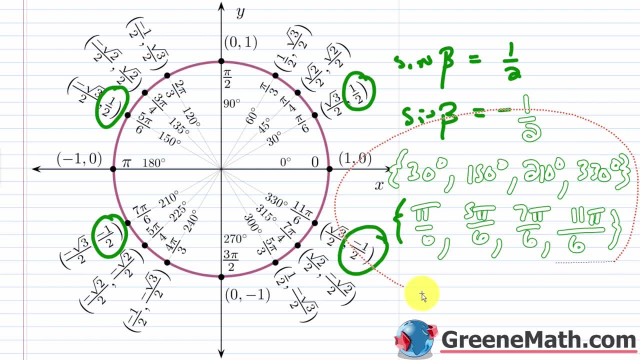 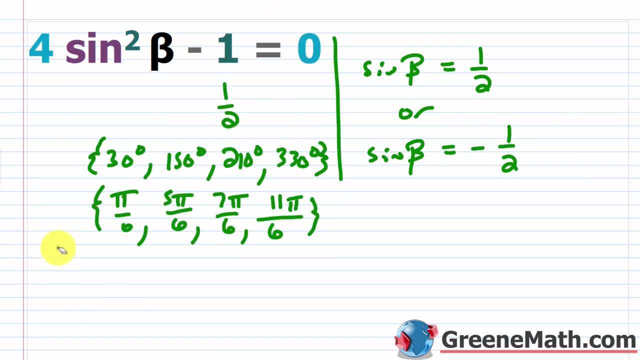 if you said between zero and two pi in terms of radians. So let's just cut this away. I'm just going to cut this. come back up here and paste this in. Okay, So these are going to be, again, our solutions. 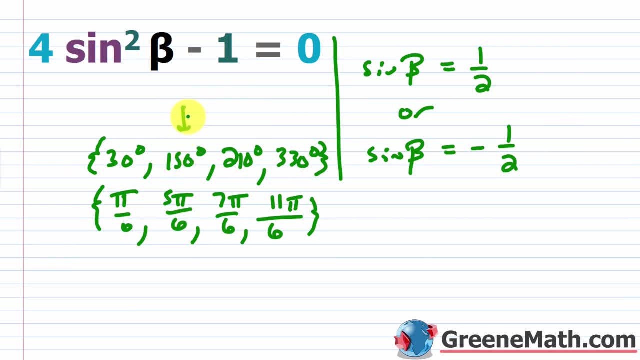 Let me just erase this Nonsense here. These are going to be our solutions, for basically, if you restricted this over an interval, again you have from zero degrees to 360 degrees- That's this guy right here. And then this guy right here would be from zero to two pi. 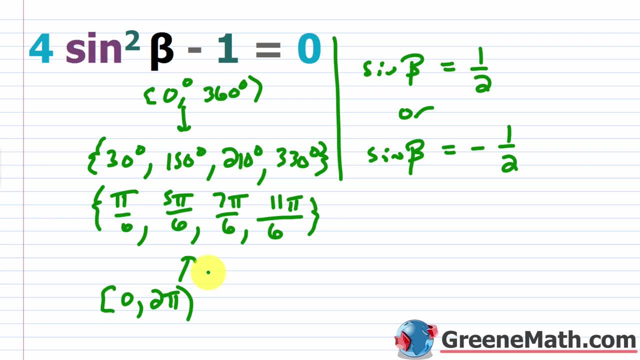 Okay. So sometimes they ask you this question to solve over a specific interval, And then other times they'll say, hey, what's the general solution? So if we want the general solution, let's just put this right here really quickly. Remember, when you work with sine, the period is going to be 360 degrees. 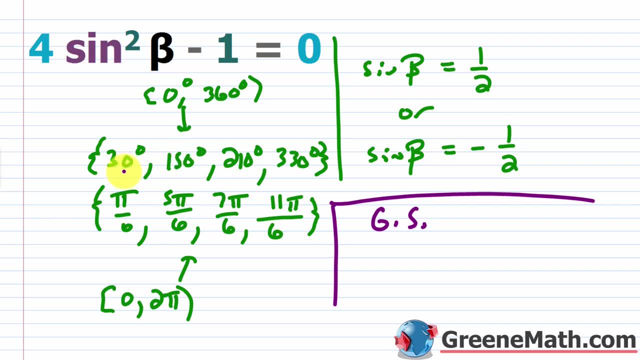 But what you notice here is that as you jump here from 30 degrees to 210 degrees, you're increasing by 180 degrees. Okay, So I would start this by saying: I have 30 degrees plus 180 degrees times some integer N, and then you'd have 150 degrees. 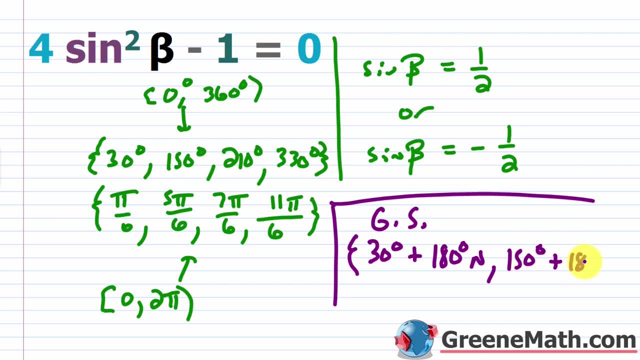 So 150 degrees plus this 180 degrees times N, because again, if you look at 150 degrees and 330 degrees, those are different by 180 degrees. Okay, And what's causing this? If we go back to the unit circle, if I circle this one again, 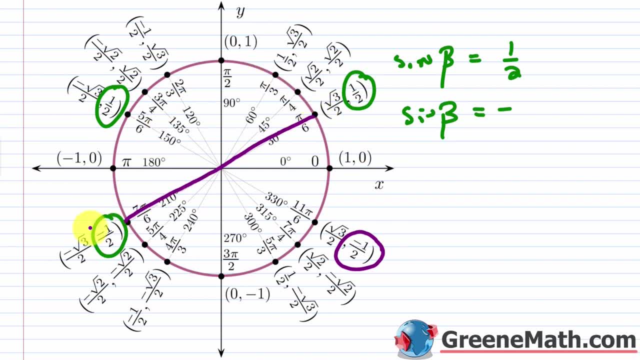 you'll notice that these guys are across from each other. This is 180 degrees, right? So, basically, these are across from each other and these are across from each other. Okay, So you can basically say that you start with 30 degrees and you add 180 degrees to get your next solution. 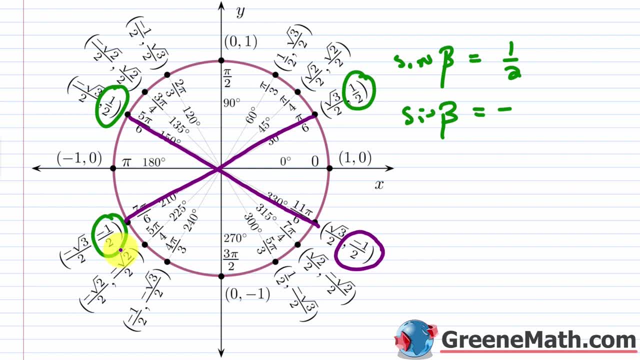 Then you add to 180 degrees again, you get to the next solution, so on and so forth. If you start with 150 degrees, you add 180 degrees to get your next solution, then 180 degrees again, so on and so forth. 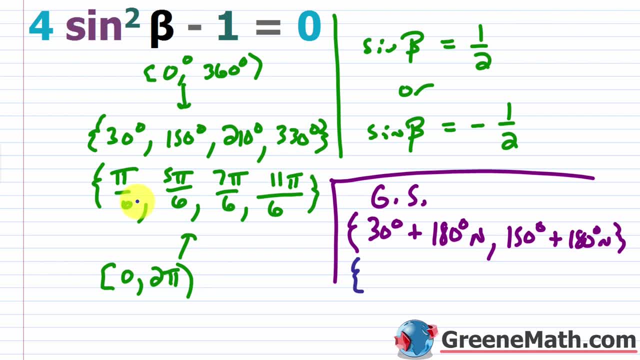 Okay, If you wanted to put this again in terms of radians, we're going to use the same concept here. I'm going to go pi over six. So basically you're 30 degrees. then plus 180 degrees in terms of radians is going to be pi. 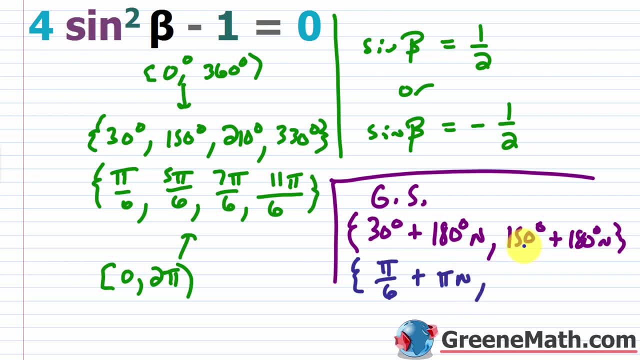 Okay, So you're just going to do pi times N And then, for 150 degrees, this is going to be five pi over six, So five pi over six, And then I'm just going to go plus my pi times N. Okay, So here's all the solutions that you could possibly want. 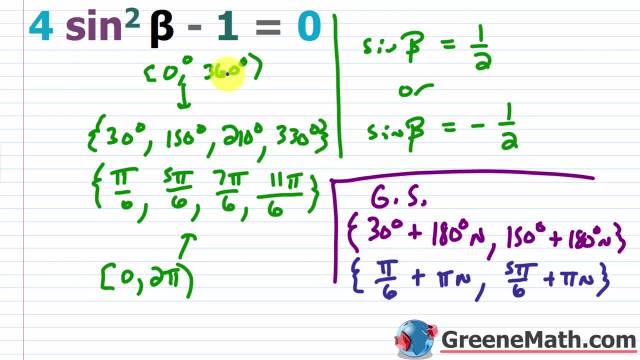 You have your degrees across that interval, from zero degrees to three. You have your radians across that interval from zero to two pi, And then you have your general solutions. So they're just basically, if they didn't ask you to solve over an interval. 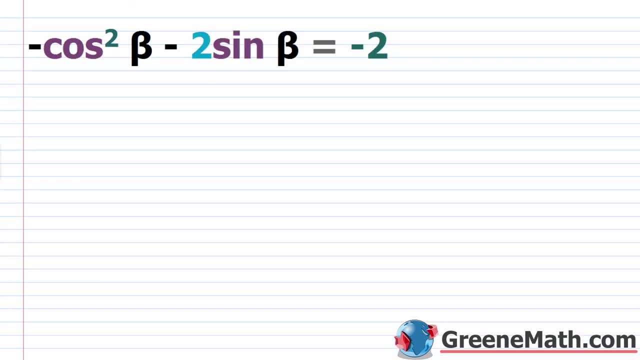 this is how you'd want to list this for degrees and then for radians. Let's take a look at another example. So here's one where we're going to need to use some identity. So we have the negative of cosine. squared beta minus two times sine of beta is. 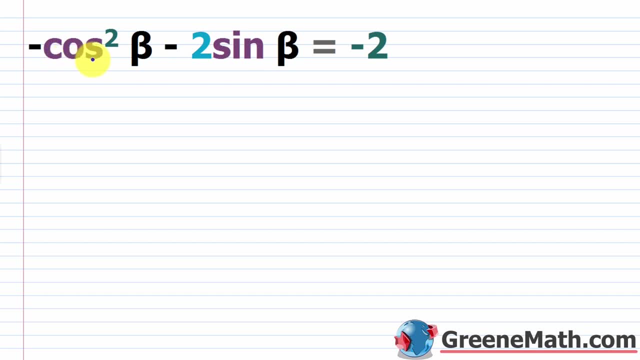 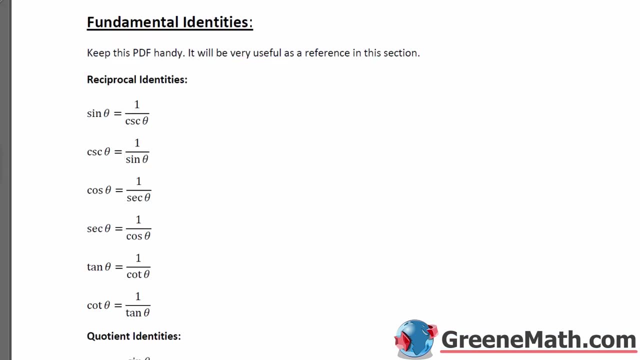 equal to negative two. So notice that you have sine here and then also cosine here, and cosine specifically a square. Okay, So what you're meant to think about if we go back to our worksheet or our little handout on the identities, if you go to the Pythagorean identities- remember, cosine squared, theta is the same. 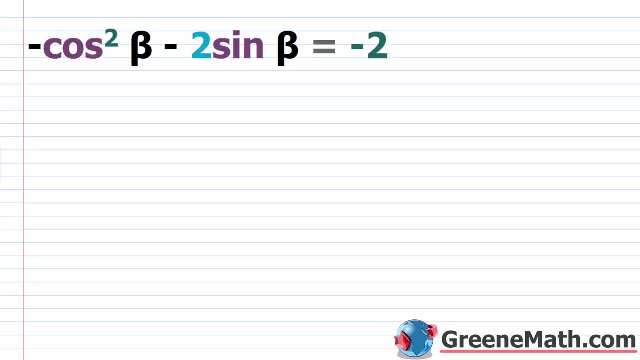 as one minus sine squared theta. Okay, So you want to look for possibilities there where you can substitute things in. So remember the negative here. This is a big deal. If you have a negative there, you're putting a negative. Put this in parentheses. 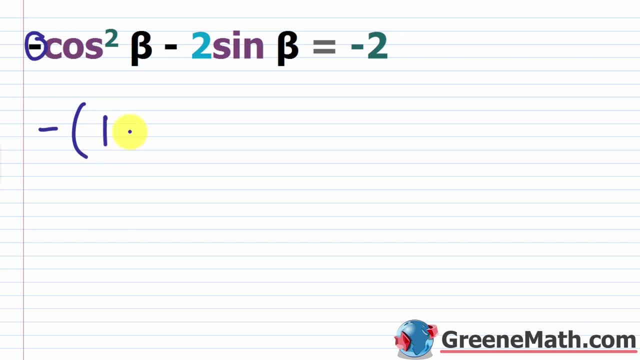 What I'm going to do, because the negatives got to get distributed to everything, So I'm going to go one minus my sine squared beta- Okay, Again, that's in parentheses. Then minus your two times your sine of beta is equal to negative two. 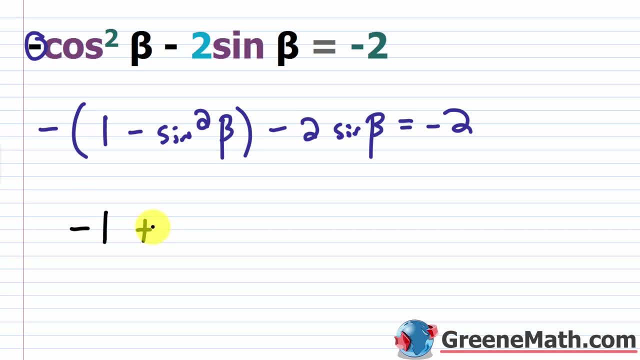 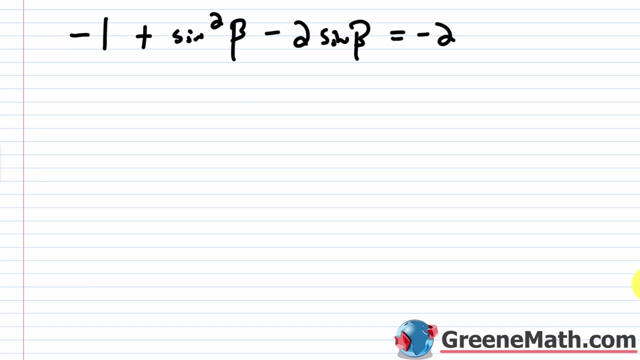 Okay, Distribute the negative to everything. So I'll say negative one, and then plus sine squared beta, Then minus two times sine of beta is equal to negative two. Okay, So from here we already know what to do We want to end up with. sine of beta equals some number, and then we want to solve. 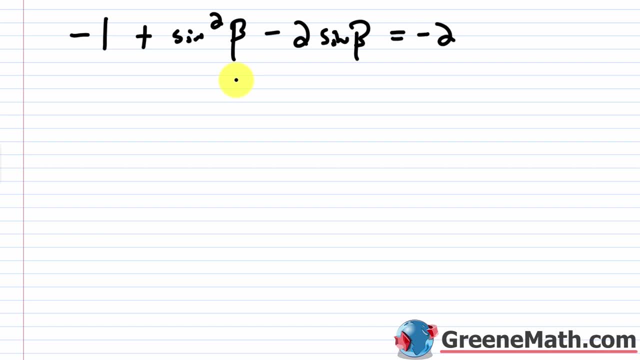 Right. So I'm going to tell you in advance: this is factorable If you have something that is quadratic in form. if it's not factorable, you can use the quadratic form. Okay, But here we're going to be able to factor. 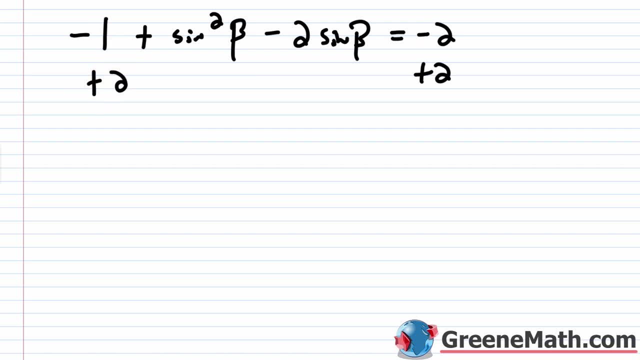 So what I'm going to do is I'm going to add two to both sides of the equation And I'm just going to rearrange things. I want the square term all the way to the left, So I'm just going to say that I have sine squared beta. 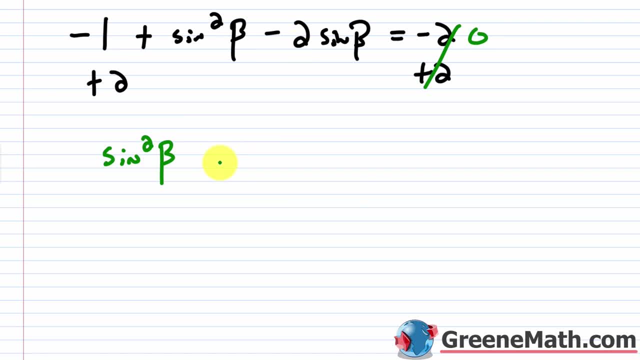 And then this is gone. I'm going to put zero here, Okay. Over here I'm going to put minus two times the sine of beta, And then, if I have negative one plus two, that's positive one, Okay, So this equals zero. 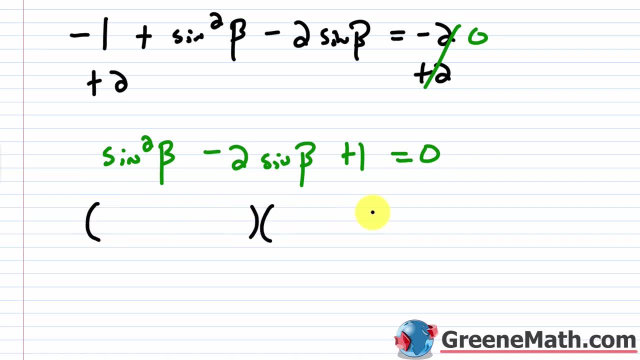 And the idea here is that I can factor the left side. Okay, So I can factor this Again. if it's a roadblock for you when you're trying to factor these guys, go ahead and take something like you and say: sine of beta equals you. 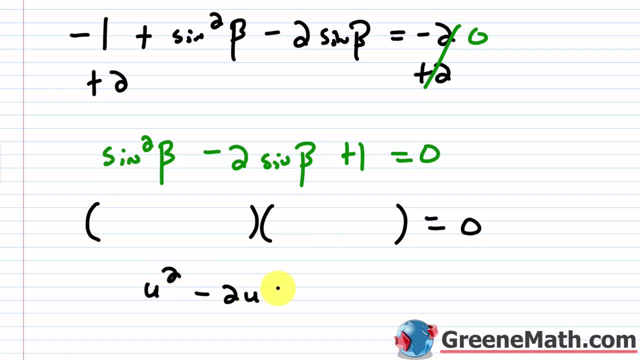 And then it's just like if you were trying to factor u squared minus two, u plus one. Okay, If that was equal to zero, you could solve that in a breeze, Right? It's just a roadblock because we're now dealing with trigonometry. 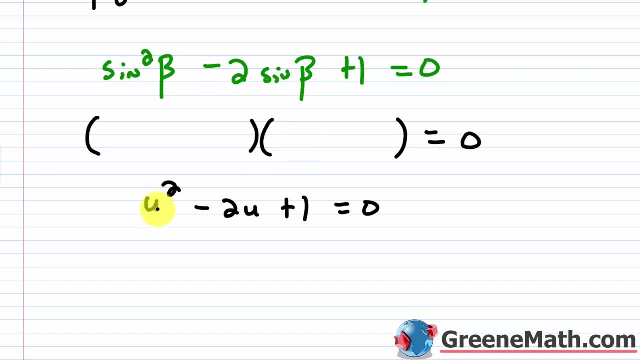 So how could we factor this guy right here And again, if it's troubling, you just look at this. Well, first off, if I had sine squared beta and there's nothing out here, there's basically a one. Well, I'm going to have. 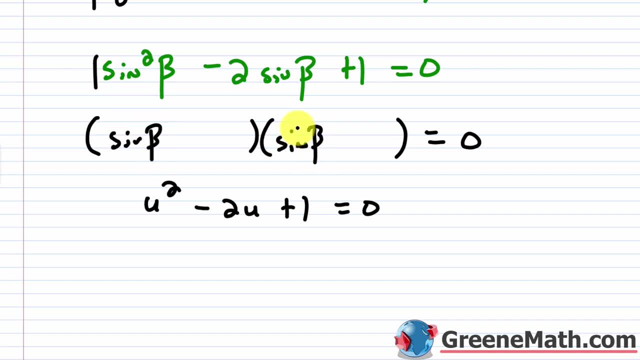 the sine of beta times the sine of beta. Okay, So that's my first term in each case. Now for this part. right here again, you're just looking at the negative two and the positive one. Okay, So I need two numbers that are going to multiply together to give me positive one. 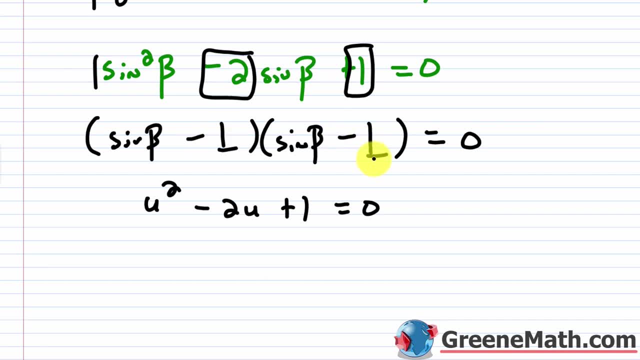 But sum to negative two. Well, that's going to be negative one and negative one. Okay, So let's go ahead and get rid of this. And basically we could write this, okay, as the sine of beta minus one quantity squared. Okay, So this equals zero. 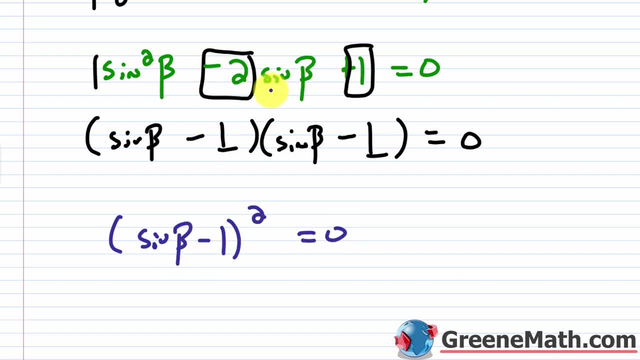 And the reason I write it like this is you can write it like this or this. Remember, this is basically from special factoring. When you think about this, it's really only going to be one of these guys that we have to set equal to zero, right. 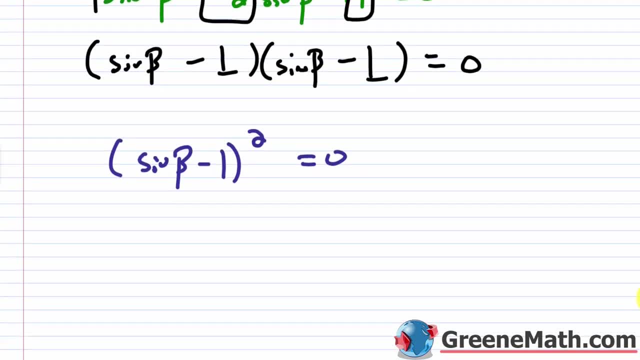 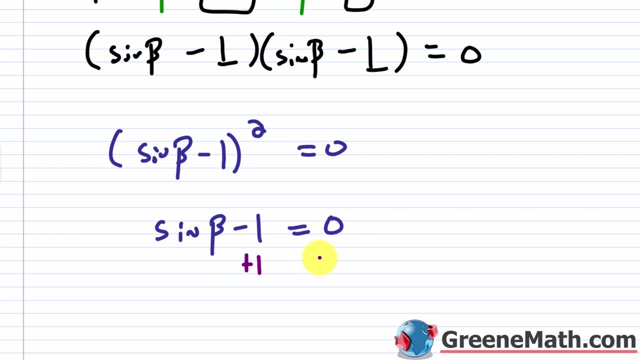 Because you have a duplicate solution. So basically, all I want to do here is just again, take one of these and say: sine of beta minus one is equal to zero. I'm going to go ahead and add one to both sides and just say the sine of beta is equal to one. 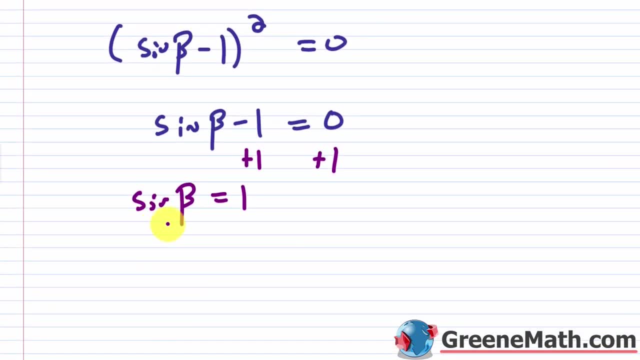 Okay, Now this is going to be really easy to solve for us. Where does the sine of beta equal one? Well, if we're looking for the sine of beta, we're looking for the sine of beta. If we're looking for the sine of beta equals one. 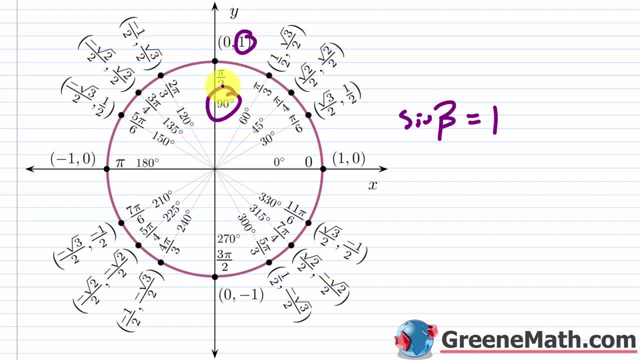 Well, again, where's the y coordinate one? Well, right here, right. So at 90 degrees, or pi over two in terms of radians, And that's basically the only place there. So your general solution would just be you rotating around another 360 degrees before you get there. 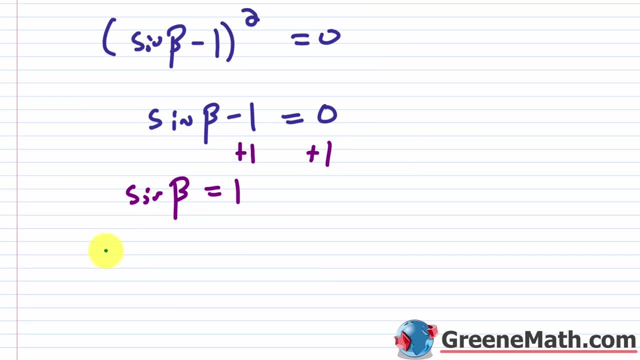 Okay, So let me go back up. So let's just put our solution here. So again, if we're in the interval, if they give you degrees, you want to answer in degrees. So if they say, over the interval you have zero degrees, and then to 360 degrees, 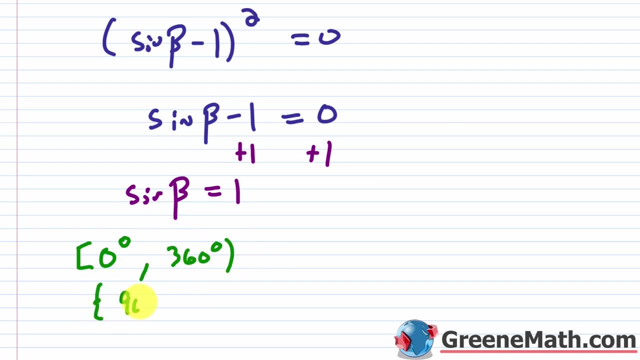 Again, if you get this, then your answer should be in degrees, And you'd want to put 90 degrees here. Okay, If you got an answer, or if you got a test question where let's say it was with radians, so let's say they said zero to two pi, like this: 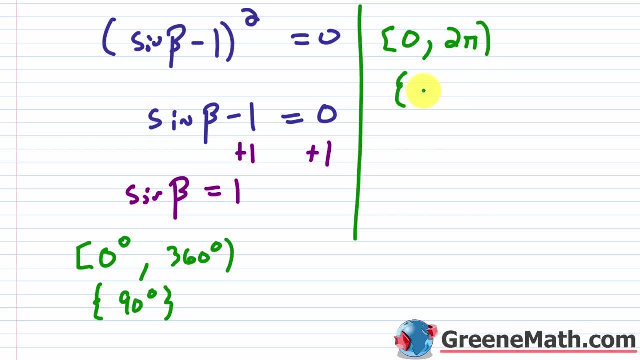 Okay, Then now you want to give your answer in radians, So you could say: beta is equal to pi over two. Or, if you do the solution set notation, just ask your teacher what they want. Okay, So I'm just going to do this. 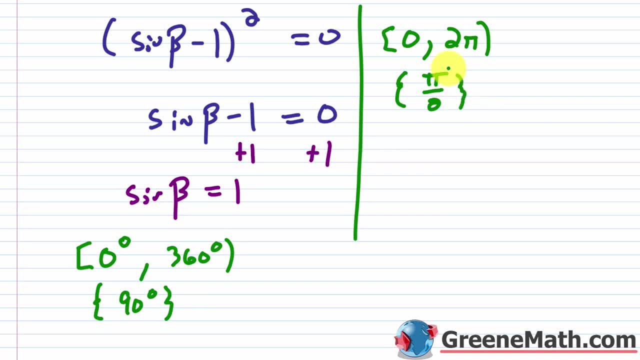 So pi over two. Okay, So that's my solution, basically in these intervals. Now again, a general solution is where we keep thinking about, when we're just keep rotating around and around and around. So basically your general solution, if it's in terms of degrees, will be 90 degrees plus another full rotation is 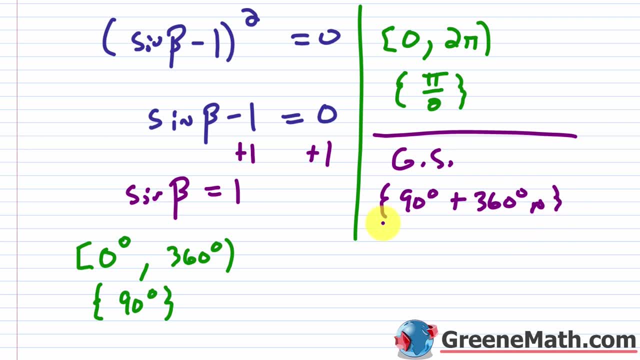 360 degrees times some integer n. Okay, And then for the radians, you just use this pi over two And then plus again, one full rotation in terms of radians is two pi. So you would do two pi and then times some integer n. 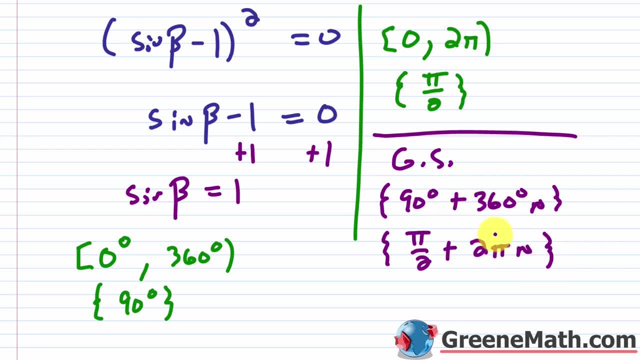 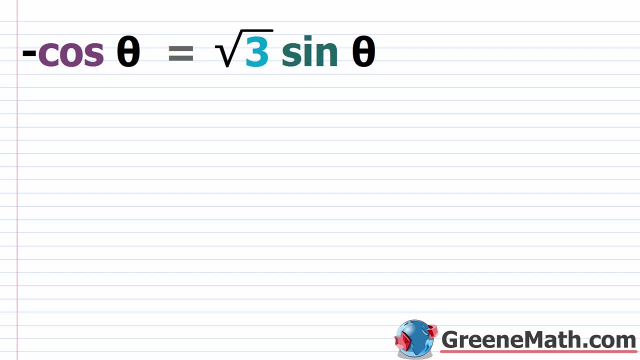 Okay, So this is your general solution here. Sometimes they ask for that, And then these are solutions If you have a specified interval. sometimes they ask for that. Okay, So let's look at a very, I would say, challenging but a very tedious type of problem. 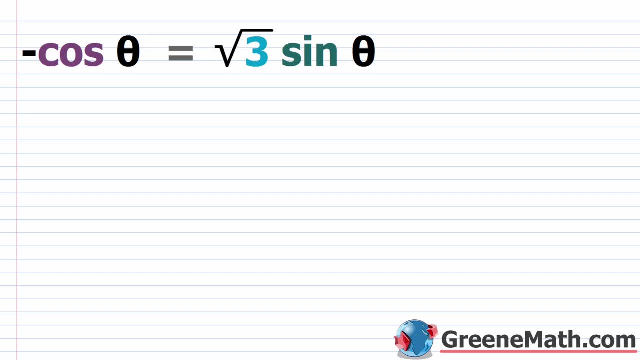 Now this one involves squaring, and you'll recall from basic algebra, If you square both sides of an equation, you lose information, And so you have to basically check your solutions in the original equation, right. You sometimes get these extraneous solutions. 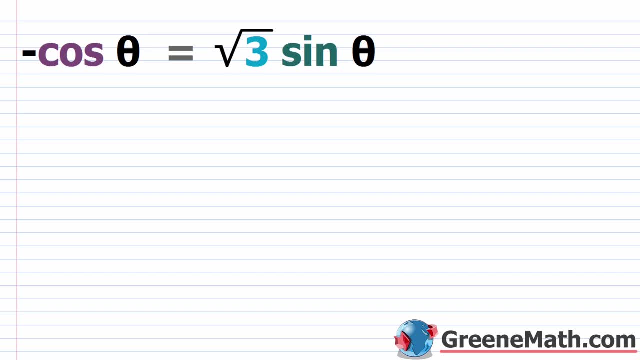 And so they're not going to work as solutions to the original equation. Okay, So we're going to see that here And we're going to see that it just takes a long time to go through everything. So the negative of cosine theta is equal to the square root of three times the sine of theta. 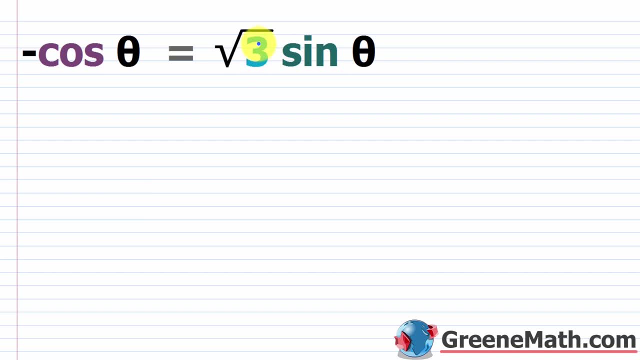 Okay. So the first thing I'm going to do is square both sides. Okay, Because I want to get rid of this radical And also I have cosine and sine, So I'm thinking Pythagorean identity. Okay, So I'm going to square both sides. 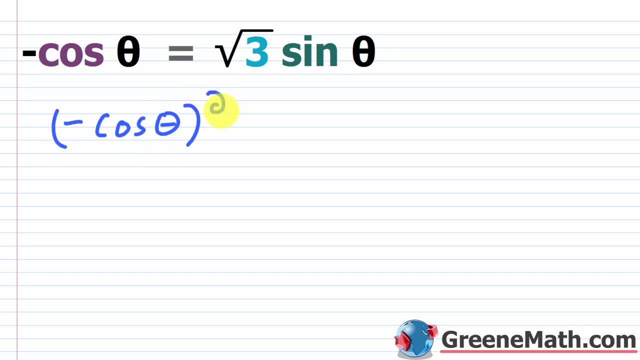 So let me write this as the negative of cosine of theta. Okay, This is going to be squared. This equals the square root of three times the sine of theta. This is going to be squared, Okay. So the negative is going to go away. 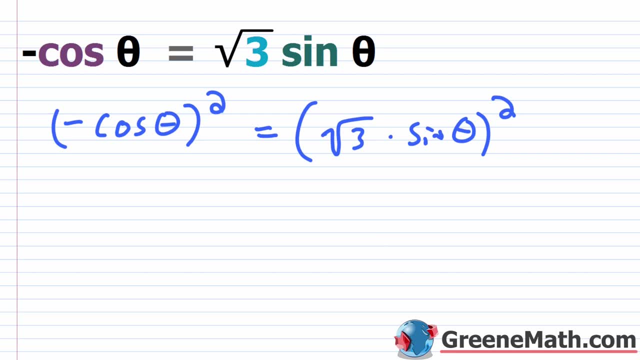 Negative squared is just going to be a positive right Negative one times negative, one is positive. So cosine of theta squared. we could just say this is cosine squared theta, like this Over here. the square root of three being squared is three. 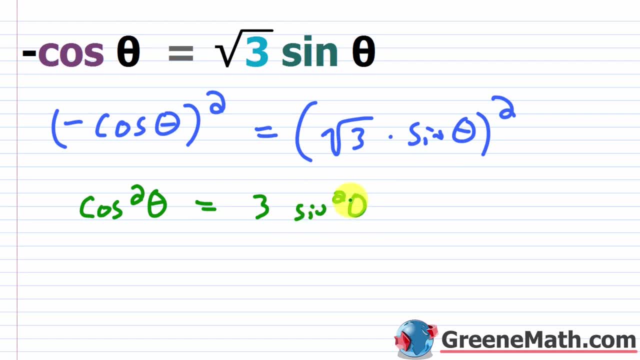 Sine of theta being squared is just sine squared theta. Okay, So at this point we know that cosine squared theta is one minus sine squared theta. Okay, So let's just go ahead and make that substitution. I'll say this: one minus sine squared theta is equal to three times sine squared theta. 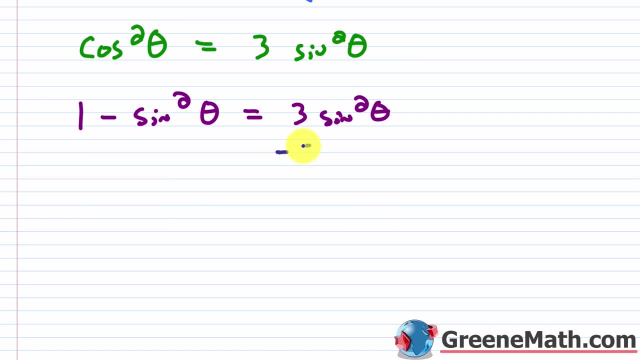 Okay, Let's scroll down and get some room going. All right, Now I'm just going to subtract three times sine squared theta from both sides of the equation And this is going to cancel, and I'm just going to put zero here. 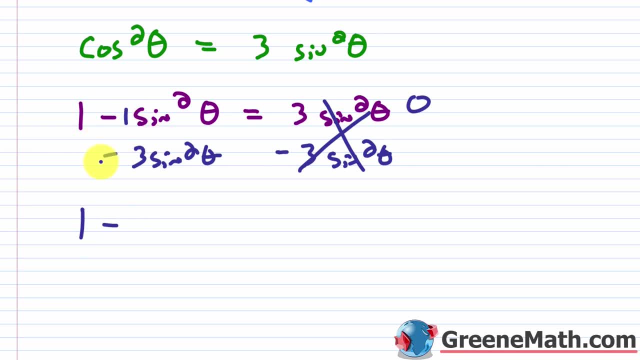 So I'm going to have one minus. Remember you can treat this as a negative one. So negative one minus three, or negative one plus negative three. However you want to think about this, This is going to be minus four. So basically, negative four times sine squared theta is equal to zero. 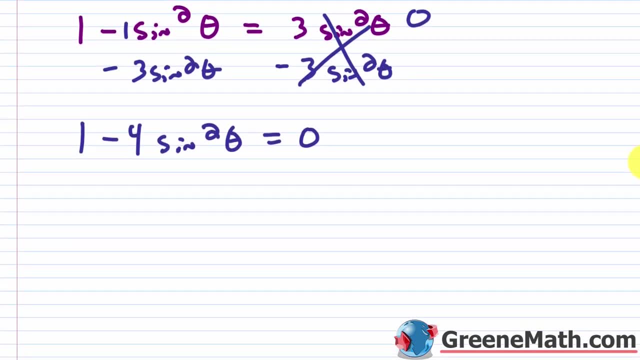 Okay. So how are we going to solve this? I want you to think back again to basic algebra. Okay, This is where your skills really come into play. Let's say it's something like a squared minus b squared. How would you factor this? 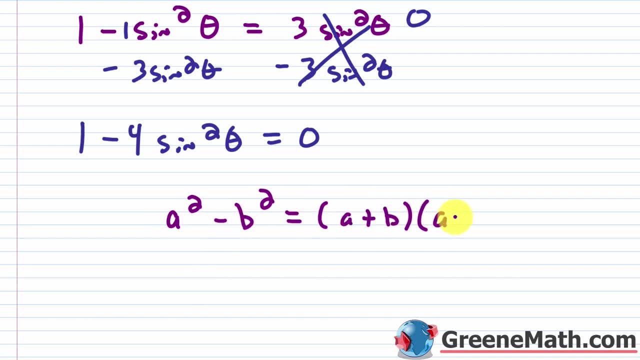 Remember, this is the difference of squares. So it's a plus b- Okay, That quantity times a minus b, that quantity. Well, here you have the difference of squares, right? I could write this out and say that this is one squared minus. you could do two times the sine of theta. 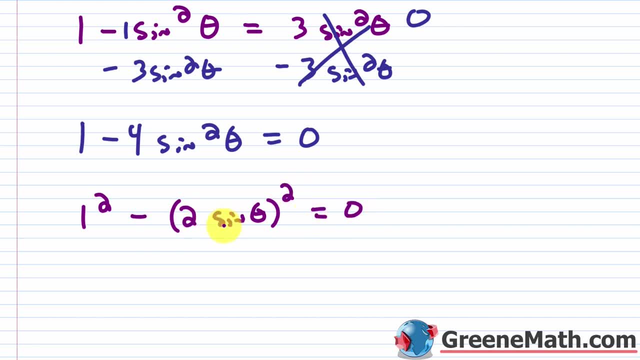 Okay, Quantity squared like this: And this equals zero. Okay, So now it's apparent, or it's very clear, that this is the difference of squares. Sometimes you have to rewrite things like that. So this would be one plus two times the sine. 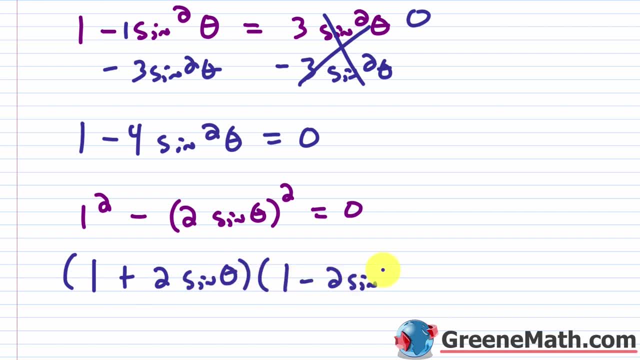 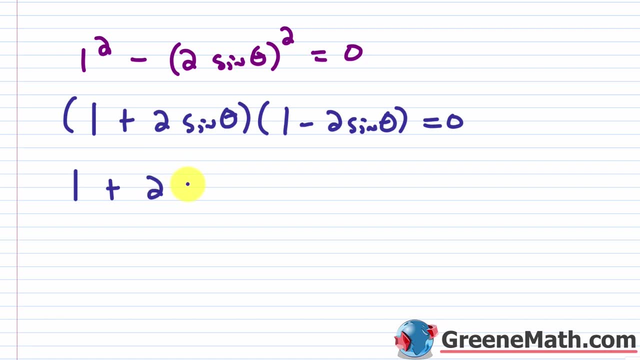 Of theta, times one minus two times the sine of theta. Okay, And we'll set this equal to zero. So basically, I'm going to take each one of these guys and set it equal to zero. So I would have one plus two times the sine of theta is equal to zero. 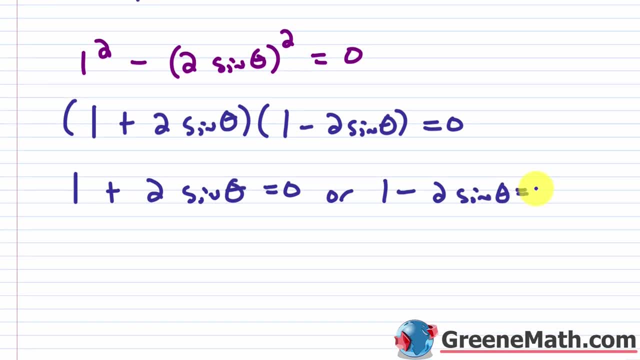 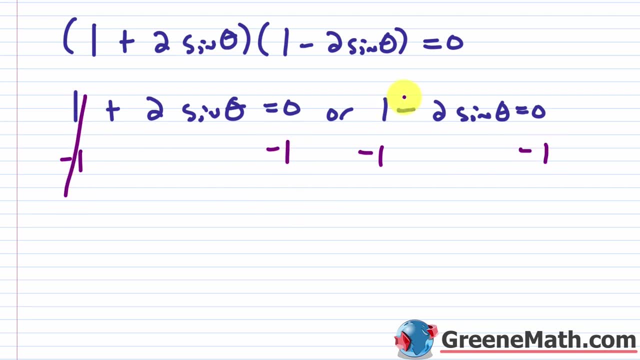 Or you'd have one minus two times the sine of theta is equal to zero. Let's go ahead and solve. They're very easy to solve. I subtract away one from each side, over here, and over here and over here, And this is going to cancel, and this is going to cancel. 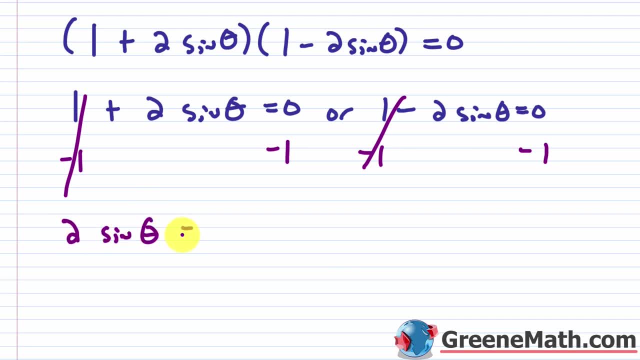 Okay, So over here I have: two times the sine of theta is equal to negative one. Over here I have only put the or I have negative. two times the sine of theta is equal to negative one. Okay, So basically at this point I'm just going to divide this by two. 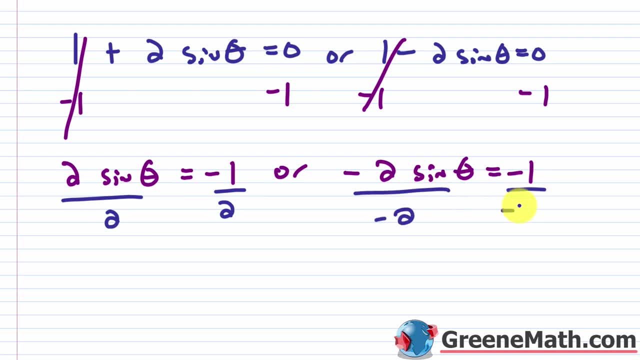 Okay, And this by two, and then this by two, or this is negative two over here and this by negative two. Okay, So this cancels, and I have sine of theta is equal to the negative one. half, Then, or over here. this is going to cancel. 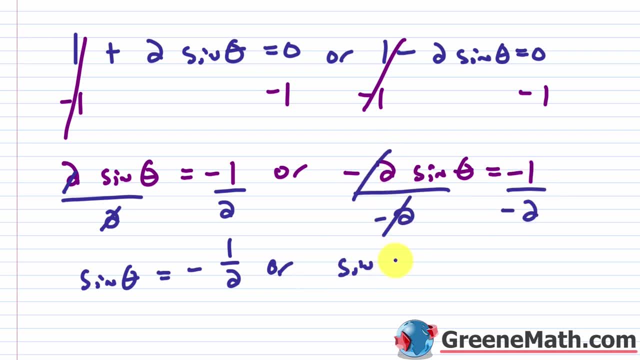 Right. And you have negative divided by negative, So that's positive. So you get: the sine of theta is equal to one half, Right? So you can condense this down and say, basically you have plus or minus one half, Okay. So let's get rid of this and let's just copy this real quick. 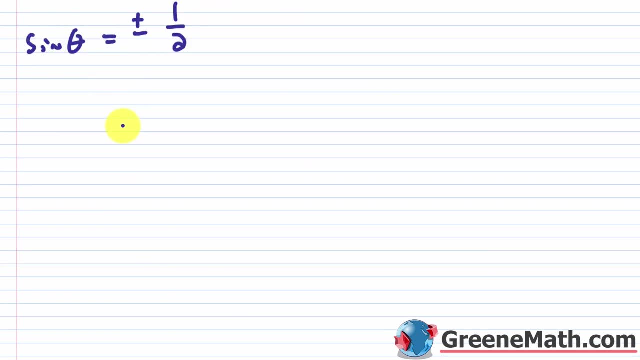 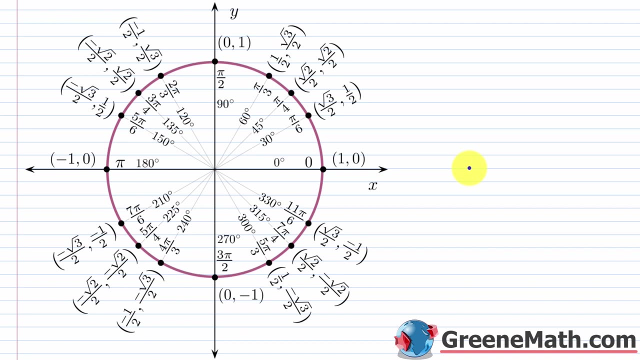 Let's go to a fresh sheet, So we have a lot of room to work, because the problem here is: you're going to get all these solutions, Okay. So if the sine of theta is a half or it's negative a half- Remember we already went through this- 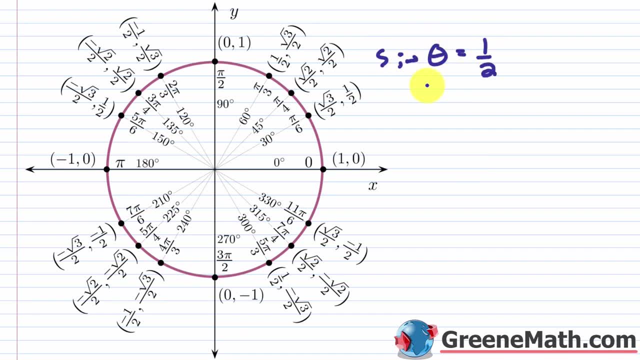 So let me write this again. So sine of theta is a half or sine of theta is negative, a half. Basically, you would have a 30 degree reference angle in each case, Right? So you would have here and then basically go around. 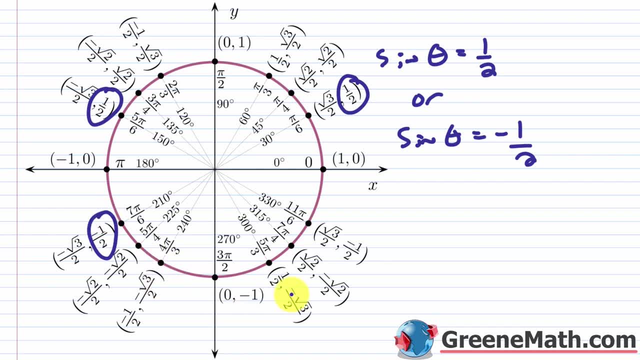 You'd have here, and then you go around and you would have right here, and then you go around and you would have right here. Okay, So we already know this, because we saw a problem with this earlier. But basically, 30 degrees, 150 degrees, 210 degrees and 330 degrees. 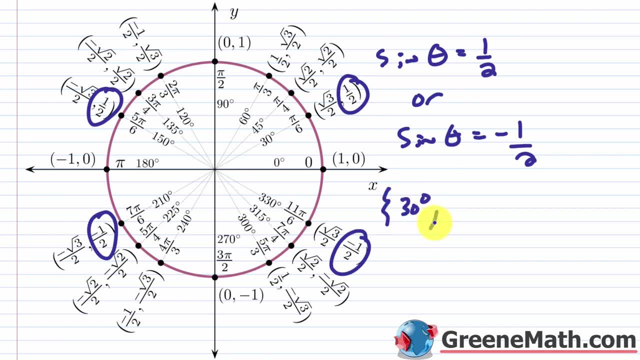 Okay, So let me write this down. So we have our 30 degrees, We have our 150 degrees, We have our 210 degrees and then we have our 330 degrees. Okay, And I'll write it in radians when we finish up. 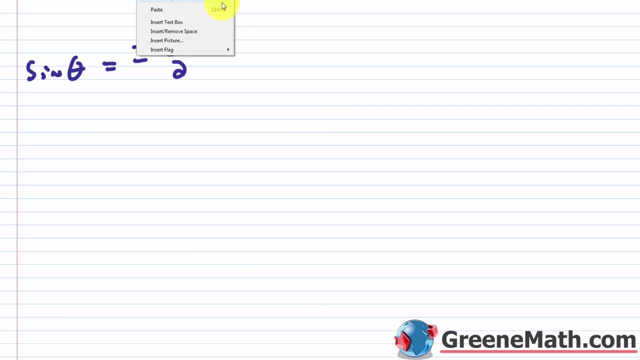 So let me just keep this in degrees for now. Let me cut this away and let me just paste this in right here. Okay, Let me get rid of all this nonsense. Now, when we square both sides of an equation, the solutions here that we get are proposed solutions. 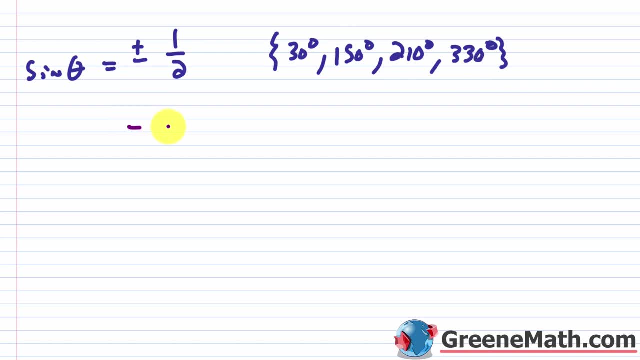 So we have to get our original equation going so we can check it. So negative cosine of theta- okay- is equal to the square root of three times the sine of theta Okay. So we're just going to use degrees. You can use radians, It doesn't matter. 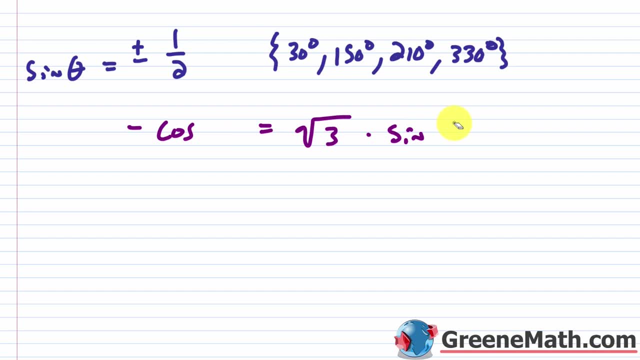 You're going to plug in for theta, Okay. So basically, if I plugged in 30 degrees here and 30 degrees here, what would we get? Well, again, I could go back and forth between the unit circle, but a lot of you already know that the sine of 30 degrees is a half. 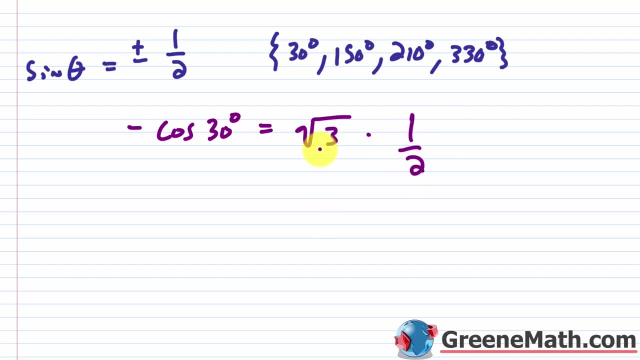 Okay, So this is going to be one half. So this would give me the square root of three over two. So let's just write that as the square root of three over two. Okay, Over here I'd have the negative of cosine of 30 degrees. 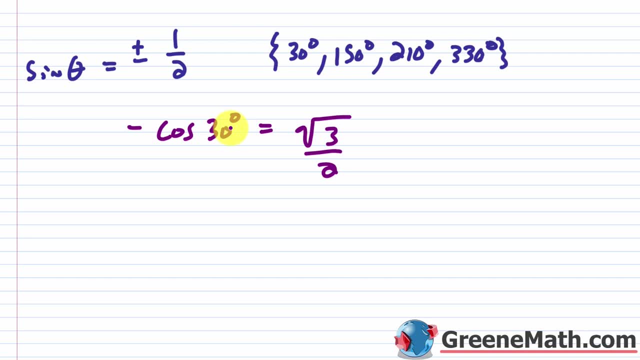 Well, the cosine of 30 degrees, you know, is a positive number, right? Because 30 degrees is in quadrant one. All of these guys are going to be positive in quadrant one, right? So there's no way this can be true, because this is the negative of a positive number. 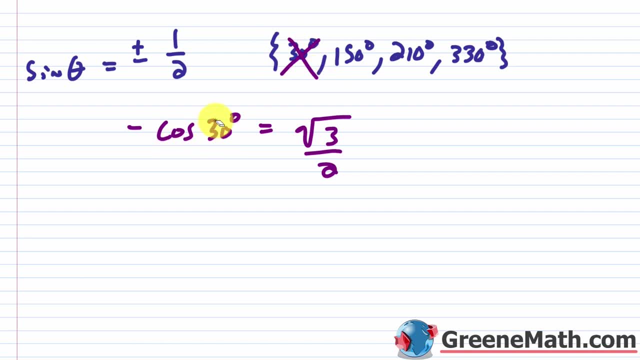 Okay, So you go ahead and mark this out. The actual answer here is square root of three over two, right, But it's the negative of that. So it's the negative of the square root of three over two is equal to the square. 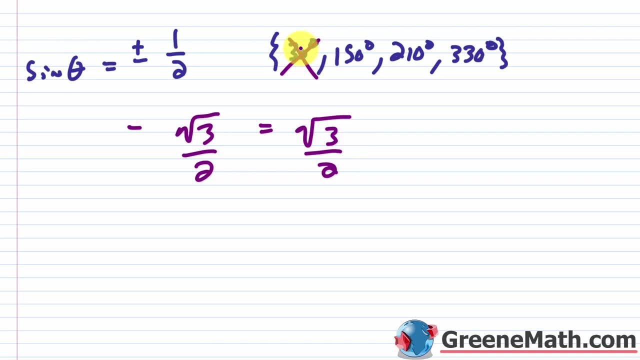 root of three over two. So that's false right. So that solution does not work. Okay, For the next one, we erase this and set this back up. So we had: the cosine, or the negative of the cosine of theta is equal to we had. 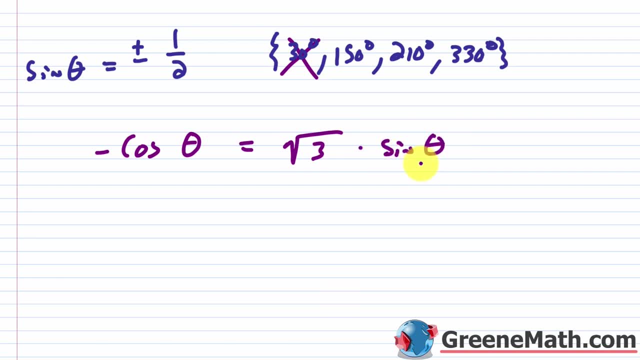 the square root of three times the sine of theta. So we know that the sine of- if I put in 150 degrees here, we know the sine of 150 degrees is basically a half right, Because the sine of 30 degrees is a half. 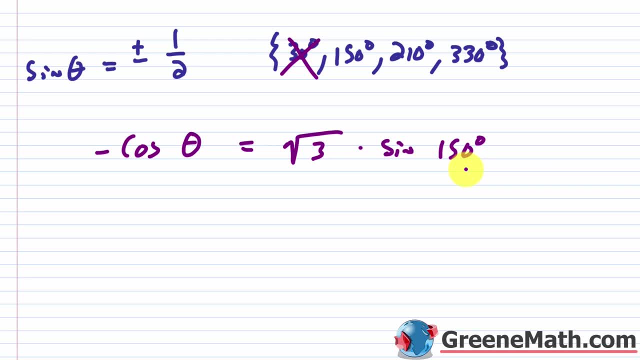 the sine of 150 degrees, because sine is positive in quadrant two. 150 degrees has a 30 degree reference angle, So this is a half as well, right? So this is basically going to be the square root of three over two. Okay, Over here, if you think about the cosine. 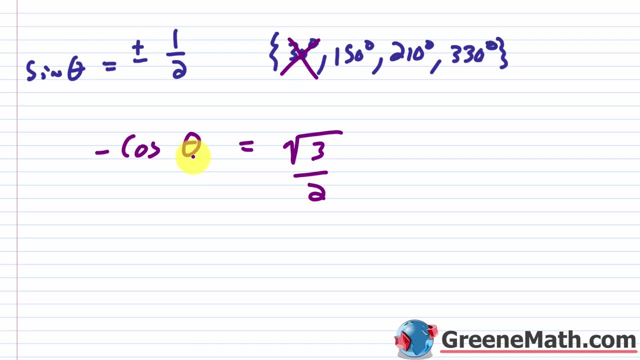 of 150 degrees. remember, cosine is negative in quadrant two. Okay, So this will save you a little bit of work. You'd have the negative of a negative which is positive. So you know this is probably going to work right. 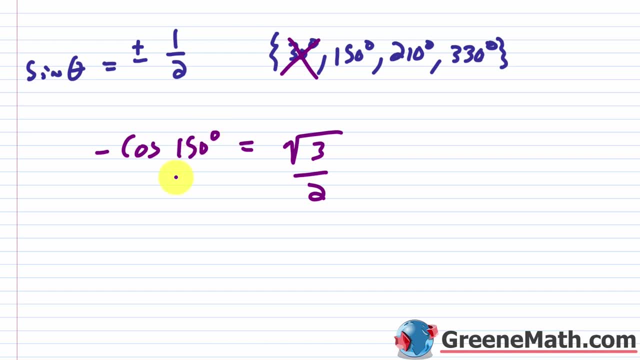 So the cosine of 150 degrees. we know that this guy is going to be the negative of the square root of three over two. Okay, But you have the negative of the negative, So be really careful. So the negative of the negative of the square root of three over two. 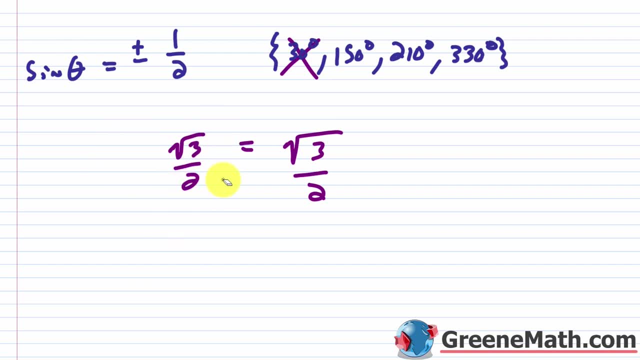 So if I apply the negative, I basically would have: the square root of three over two is equal to the square root of three over two. Okay, So this one checks out. So 150 degrees is a valid solution. Then for 210 degrees, let's go and set this back up. 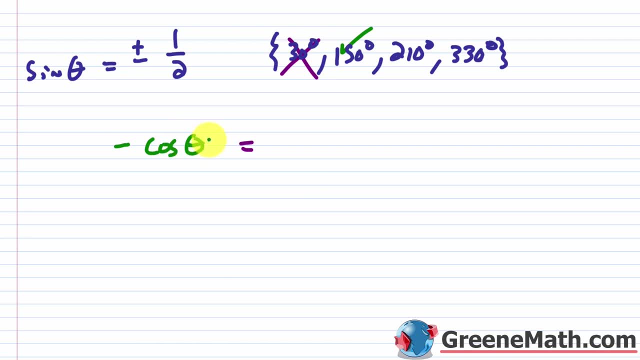 And I probably shouldn't erase this each time, But it's the negative of the cosine of theta is equal to the square root of three times the sine of theta, So 210 degrees. If you put this in here, okay, and you put this in here again. 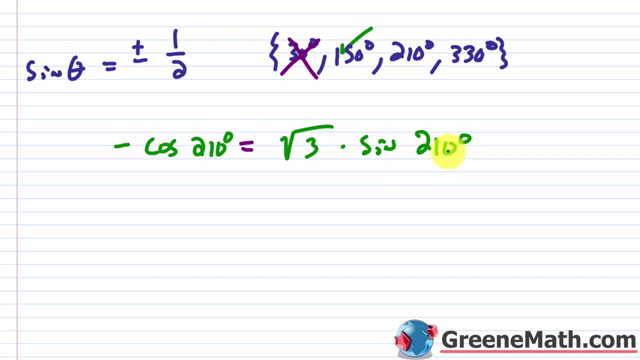 we know that the reference angle is 30 degrees, right? So what is the sine of 30 degrees? Well, it's going to be one half, But we're in quadrant three now, so we know this is negative. So, basically, this is negative one half. 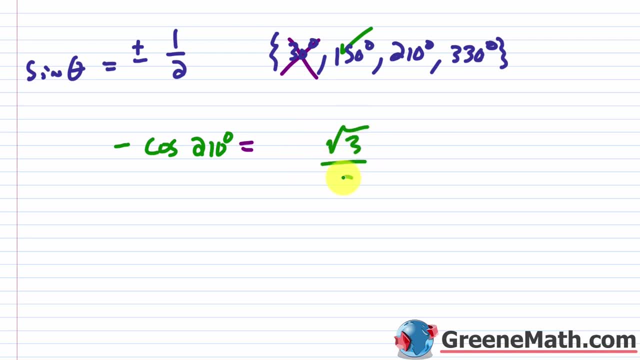 So this would be the square root of three times negative one half. So square root of three over two And this is negative. Okay, So over here 210, again, this many degrees. I know that I have a reference angle of 30 degrees. 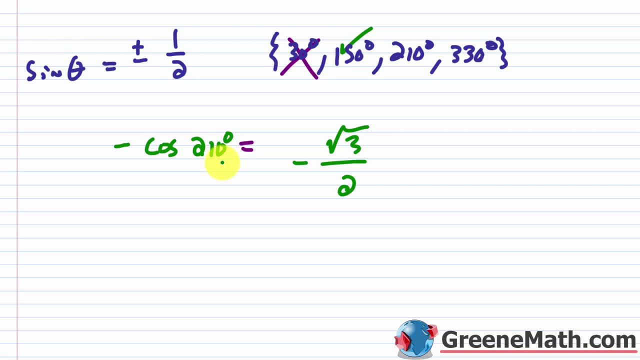 So the cosine of 30 degrees is square root of three over two And because this guy's in quadrant three cosine is negative, So this is the negative of the square root of three over two. So this isn't going to work out right. 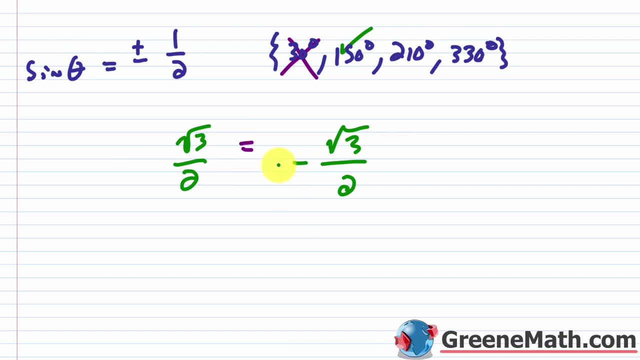 Because again, if I apply the negative, this becomes positive. So again we have one that doesn't work, So this one doesn't work, And then for 330 degrees, let me just do this one last one. So the negative of cosine. 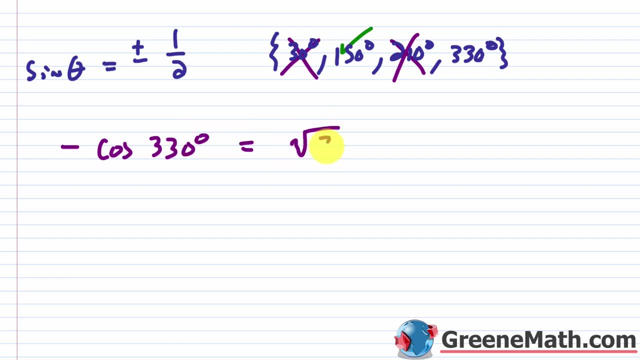 of- let's just go and say 330 degrees is equal to you have the square root of three times your sine of 330 degrees. Again I've got a 30 degree reference angle and I'm in quadrant four. So I know this is negative one half right. 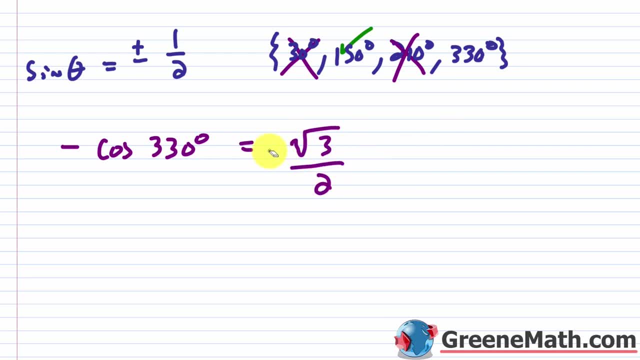 So might as well just put negative square to three over two, Okay, Like this, And I'll just put this out here: Okay, So over here again, I have a 30 degree reference angle, but cosine is positive. okay, in quadrant four. 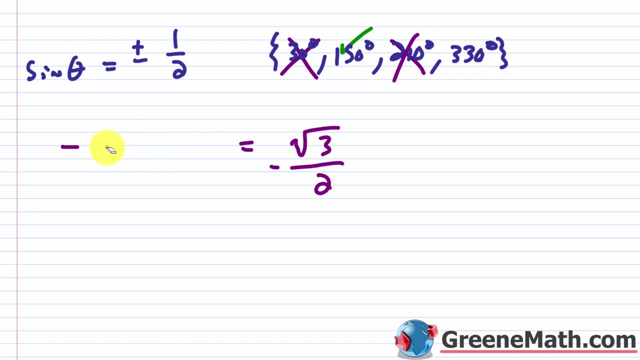 So I would say square root of three over two. So square root of three over two. But it's the negative of that, because I've got this negative hanging out. So these guys are equal, So this one does work out, Okay. So your two valid solutions here are 150 degrees or 330 degrees. 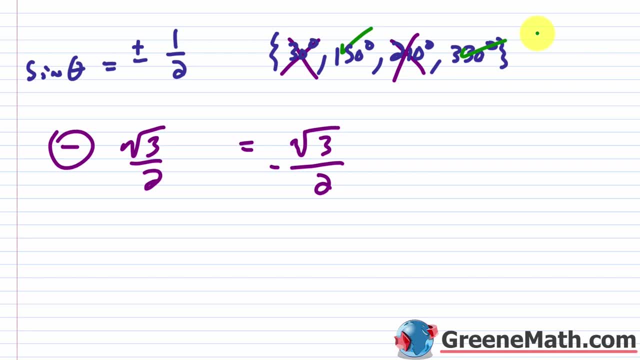 Okay In terms of degrees, And then, if you're working with radians, it's five pi over six or then 11 pi over six. So let's go ahead and write our solution here. We'll say from the interval: if you're in this interval, zero degrees. 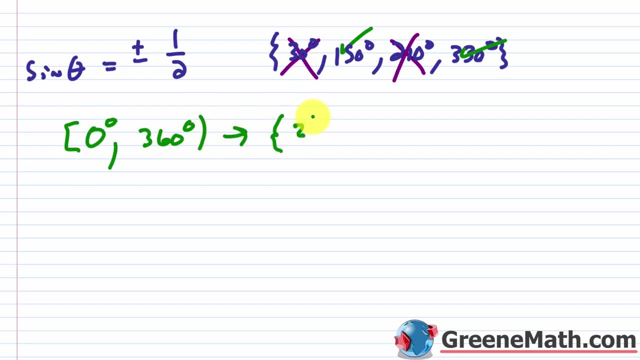 and then 360 degrees. we'll say the solution set is basically: 150 degrees Okay, And then 330 degrees only Okay. So just those two guys And then, if I'm in this interval from zero to two pi, if they give it to you like this: 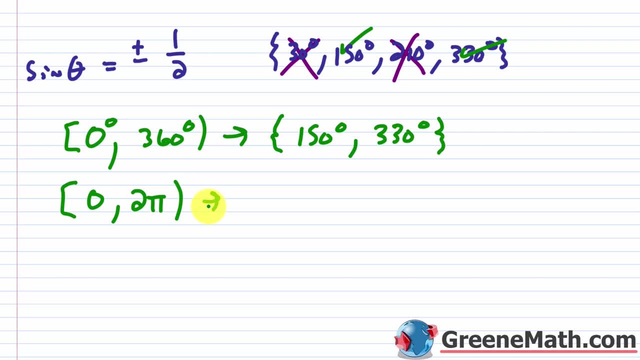 always answer based on what they give you as the interval. Okay, If they don't give you anything, then you can just ask your teacher like: hey, what do you want this in? So basically, at this point I want to do my radians. 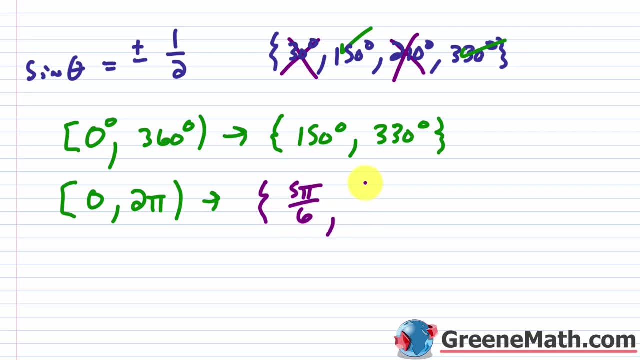 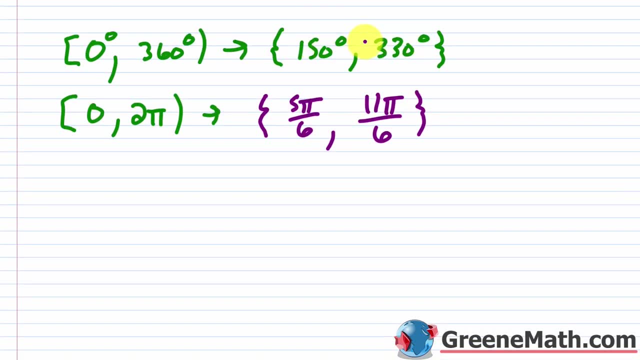 So I'll go ahead and say that this is five pi over six and then 11 pi over six. Let me close that down. And then again, if you want a general solution, you want to realize here that you can just add 180 degrees each time. 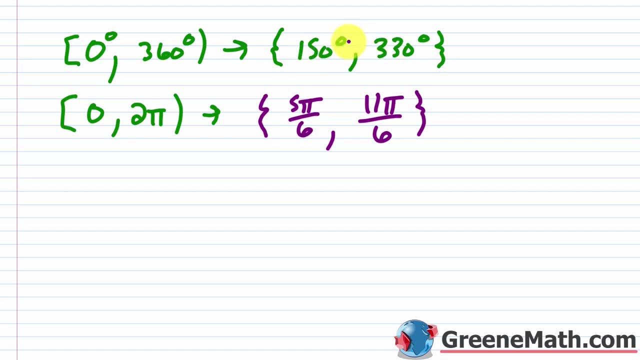 Again, I know the period for sine is 360 degrees, but you have to pay attention to this type of stuff if you're writing a general solution. So the general solution here would be: let's go ahead and say 150 degrees plus 180 degrees times that. 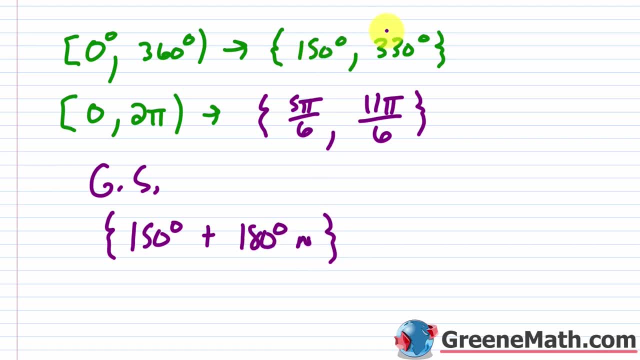 Okay, So you don't want to do 360 degrees there, because again, if I add 180 degrees I get to 330 degrees, And if I add 180 degrees to that I'm going to be at 150 degrees plus 360 degrees, which is 510 degrees. 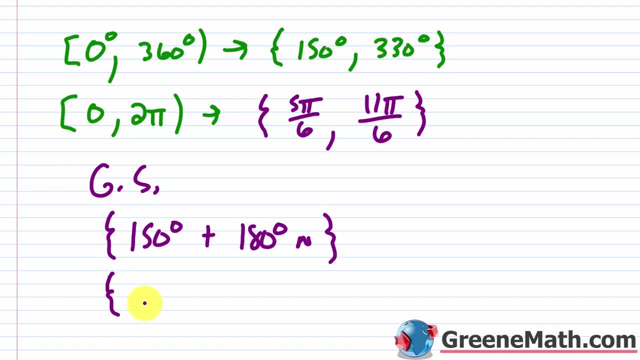 You know so on. So I'm going to go for it, Okay. And then, in terms of radians, I'm going to go ahead and say that it's five pi over six plus 180 degrees is going to be pi radians, and then times that. 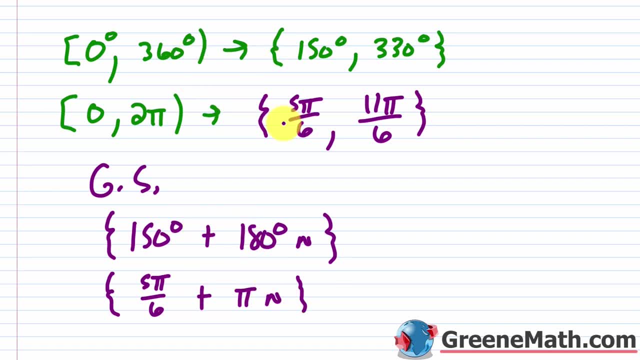 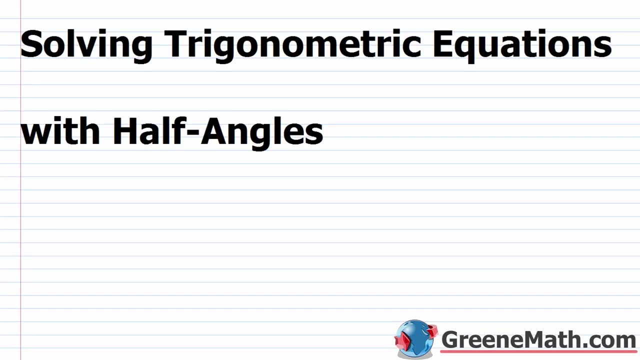 Okay, So these are your general solutions And then these are your solutions. If you're given a specific interval to solve over, just get with your teacher in terms of what you need to do. in this lesson, We want to talk about solving trigonometric equations with half angles. 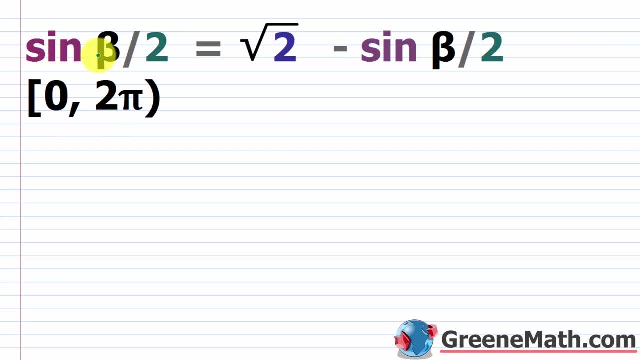 All right. So let's start off with a very easy example. So we have: the sine of beta over two is equal to zero to two. minus the sine of beta over two, We have a little domain restriction. or you could say you're solving over an interval. 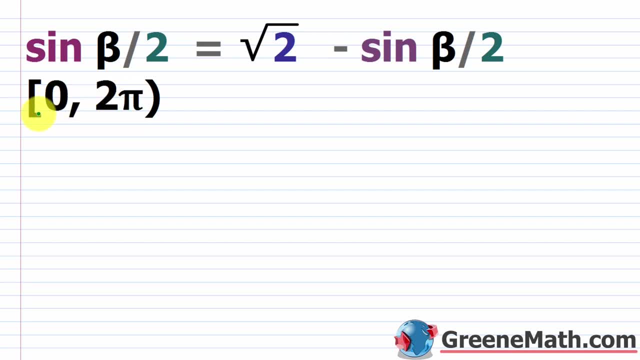 In this case it's from zero to two pi, with zero being included. Okay, Now I want to make something perfectly clear. You are solving for beta, Okay, So you want to plug something in here for beta. So basically, here and here, and you want the result of this to be true. 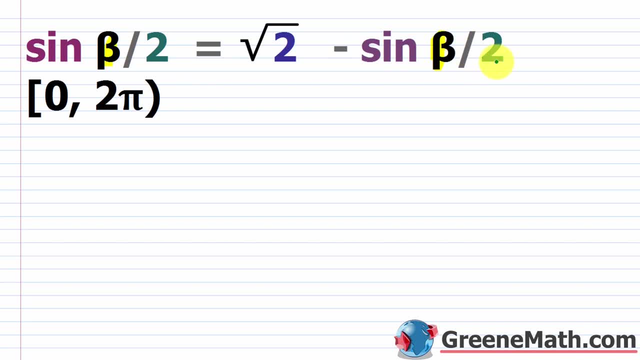 Okay, You are not, in the end, solving for beta over two, But we need to use beta over two in order to get a solution, Okay, So what we're going to have to do- and let me write this down here- I'll show you. 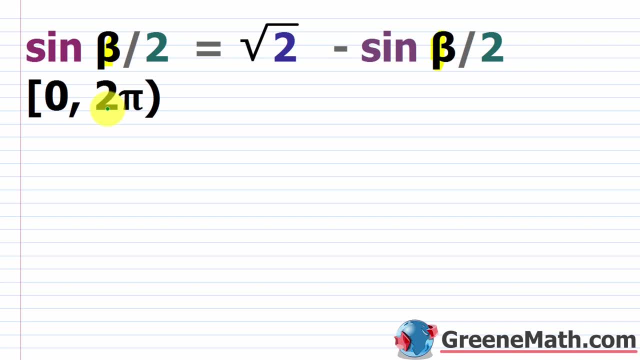 We need to basically change this up just a little bit, and I'll explain why. So let me rewrite this real fast. I'm going to say that I have: the sine of beta over two is equal to the square root of two, minus the sine of beta over two. 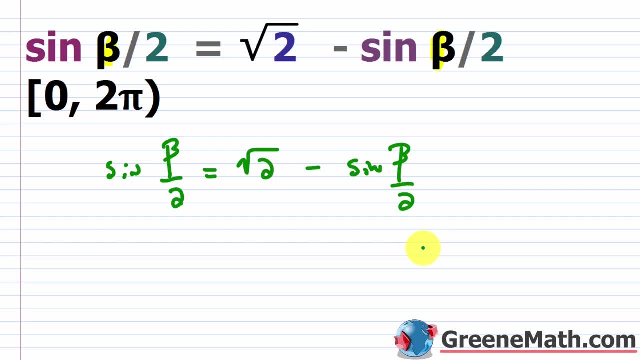 Okay. So the first thing I'd want to do is get that trigonometric expression by itself, and in order to do that, I'm just going to add the sine of beta over two to both sides of the equation. Okay, So that's how I'm going to get things started. 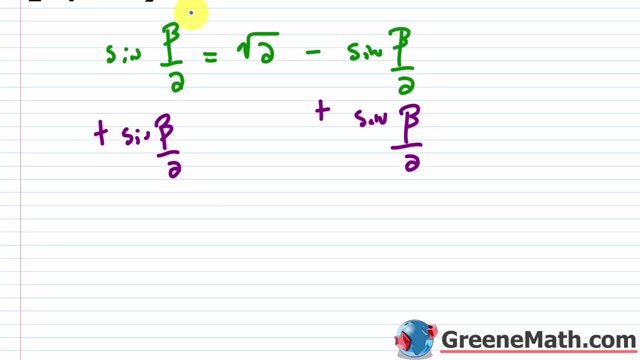 So let me scroll down A little bit here, get some room going, and I'm just going to show this cancels over here. So sine of beta over two plus sine of beta over two is two times the sine of beta over two. 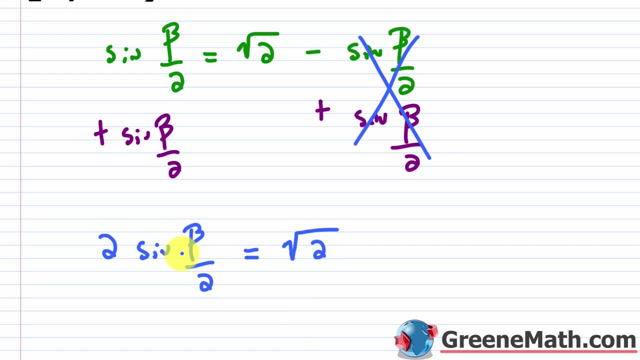 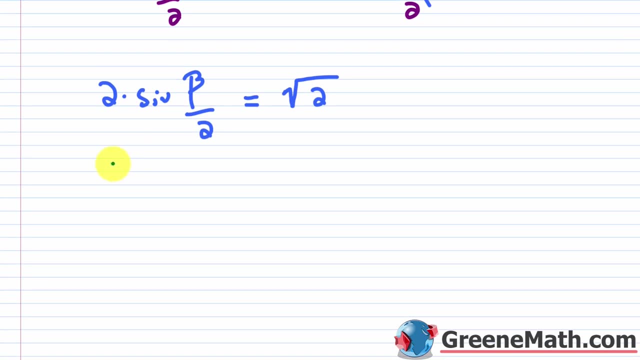 And this equals now the square root of two. Okay, If I want to isolate this completely, I'm multiplying this by two. Okay, So I can just divide both sides by two, and then I'll take care of that. So I'll divide this side by two and this side by two. 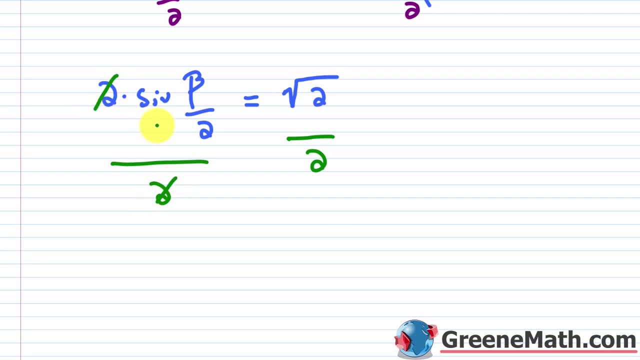 And basically this is going to cancel with this. Okay, So that's gone And I've isolated the sine And let me make that a little bit better. So it's the sine of beta over two. So that's on my left side. 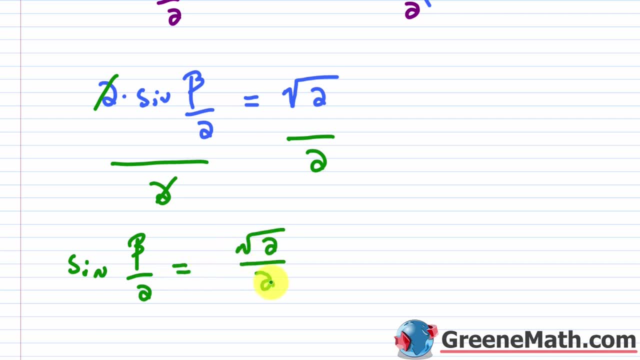 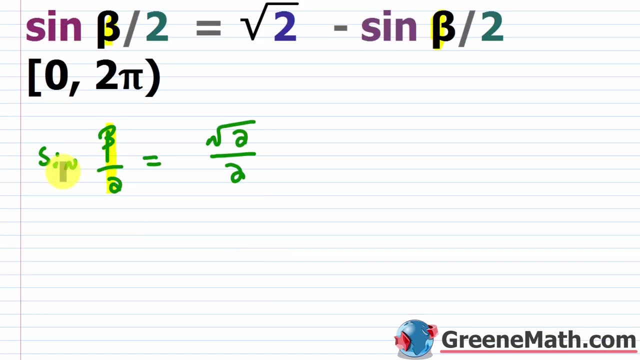 On the right side, I have the square root of two over two. Okay, So let's pause for a minute- I'm actually going to erase all this- and let's think about what we have. We have this right here, which is beta over two. 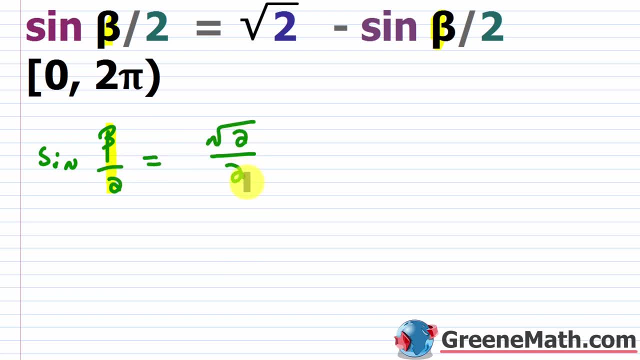 And we have the sine of that guy And we're saying that it's equal to the square root of two over two. So before we start thinking about how we're going to solve this, let's first modify our little domain to work with what we're working with here. 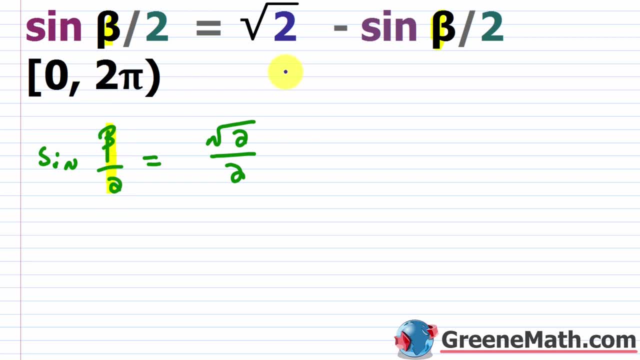 We're working with beta over two, So I'm going to write this as an inequality. I'm going to say that zero is less than or equal to. I'm going to do this beta guy here, which is less than two pi. Okay. 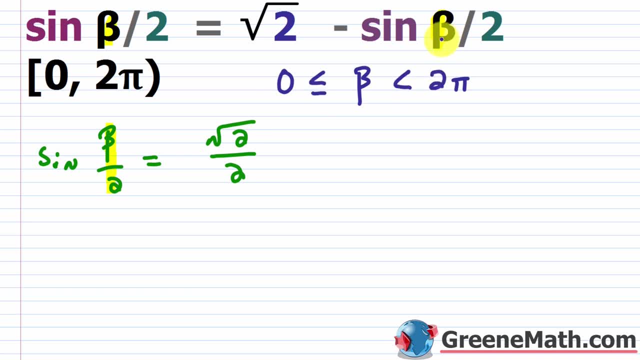 Because that's what we're initially working with. Again, this is for beta. So now we have beta over two, So we divide everything by two here. Okay, To consider the interval here. So this is just going to be zero. This will be beta over two. 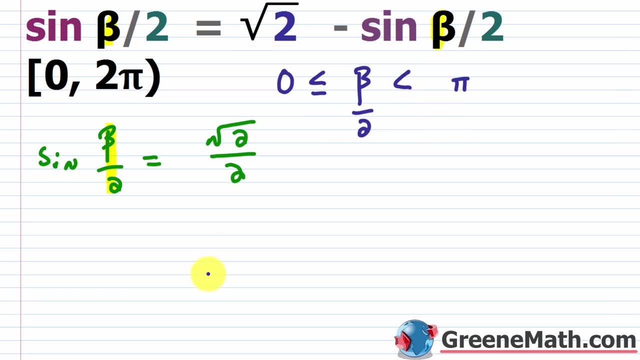 And this is just going to be pi Okay. So essentially, what I'm looking for here is I'm looking for where beta over two sine of that guy would be square root of two over two. Now, in this particular case, if you think about square root of two over two in terms of sine, 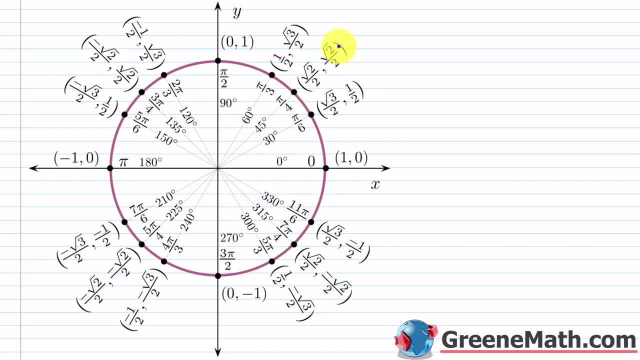 if you go to your unit circle, you can see in quadrant one you have square root of two over two here, with pi over four in terms of radians, or forty five degrees with degrees, and then you would want a forty five degree reference angle in quadrant two. 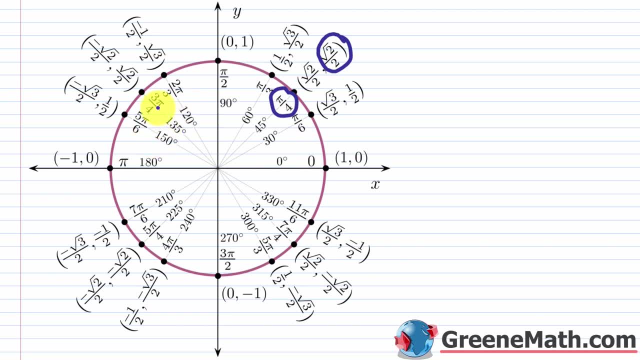 Okay. So in terms of degrees, that's going to be one hundred thirty five degrees, or three pi over four. in terms of radians: Right. So, right here, Okay, And you can see this right here. Okay, So that's pretty obvious. 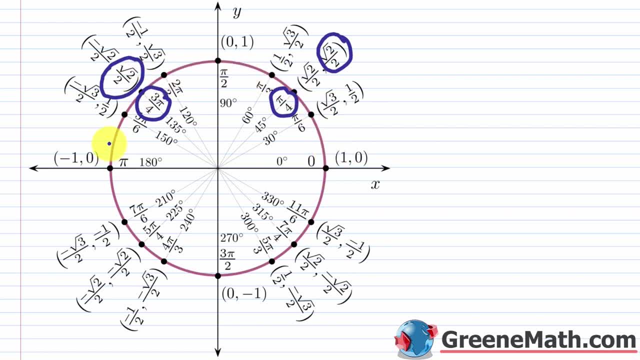 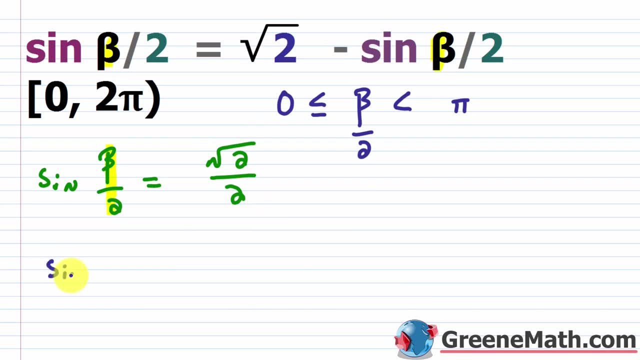 And you can see that that's falls in line with our interval for beta over two, because it's from zero to pi. Okay, So we're going to take pi over four and three pi over four. So I'm going to say that the sine of pi. 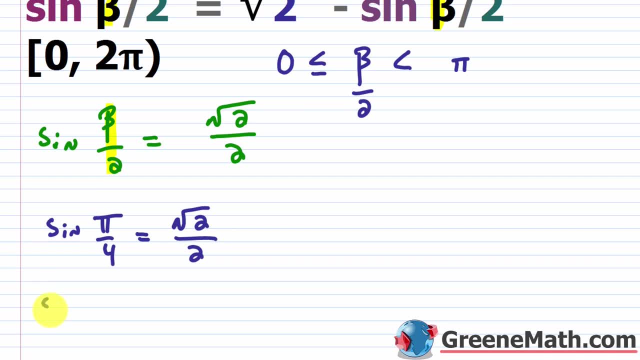 over four is equal to the square root of two over two, And also that the sine of three pi over four is equal to the square root of two over two. Okay, So what I want to think about here, now that I have everything set up, remember, you can set these guys equal. 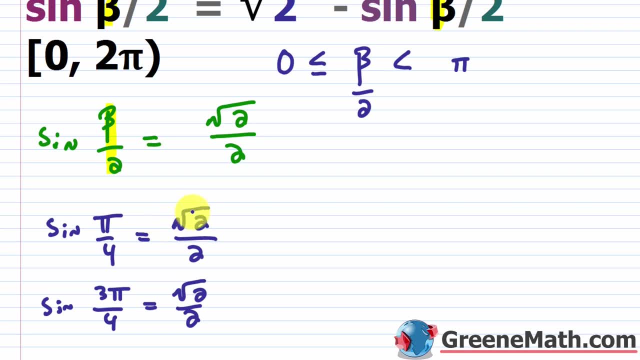 to each other, because I know that the sine of pi over four is equal to the square root of two over two, And I know that beta over two sine of that guy is equal to the square root of two over two. So what I can do here is set up a little. 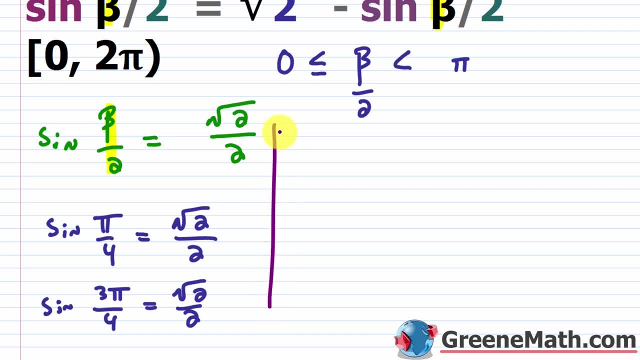 equation so that I can solve for beta, Right? So let me do this over here. I'm going to say that beta over two is going to be equal to pi over four, Because, again, sine of this guy produces this and sine of this guy produces this. 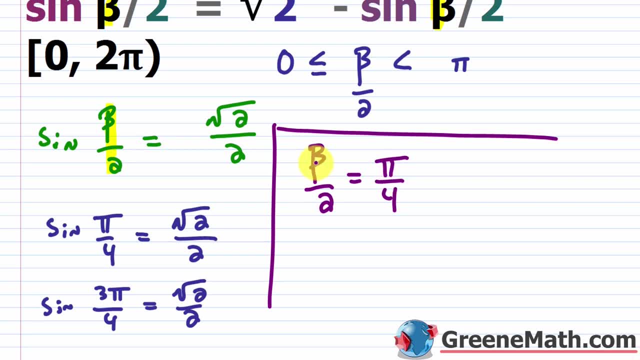 So I can set these two equal to each other in order to get a solution for beta. Okay, So that's why that's going on. Okay, So let's scroll down just a little bit to get some room. I'm going to put, or here: 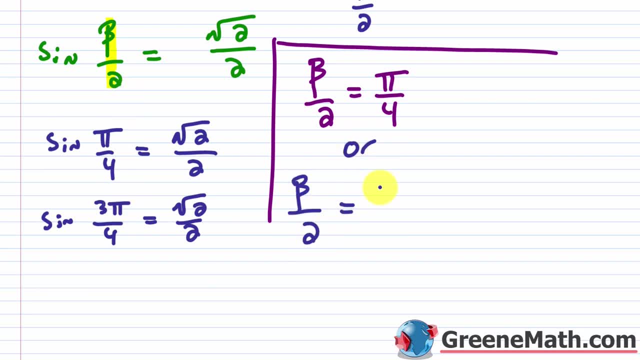 I'm going to do the same thing with this. So beta over two is equal to the three, pi over four. Okay, And all I need to do here? it's very simple to get a solution. I'm just going to end up multiplying both sides by two. 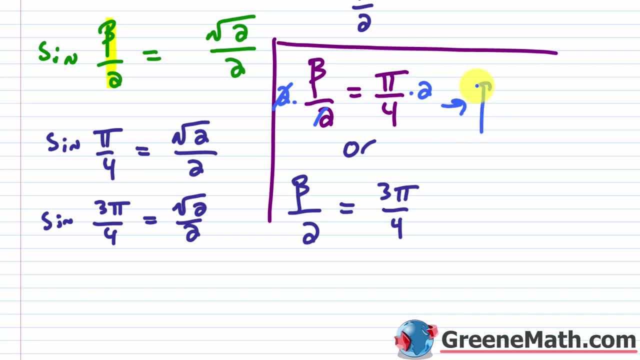 Okay, So this is basically going to be what this is going to cancel. I'll have: beta is equal to the two. would cancel the four and give me two down here. So pi over two And then over here. basically I'm multiplying both sides by two. 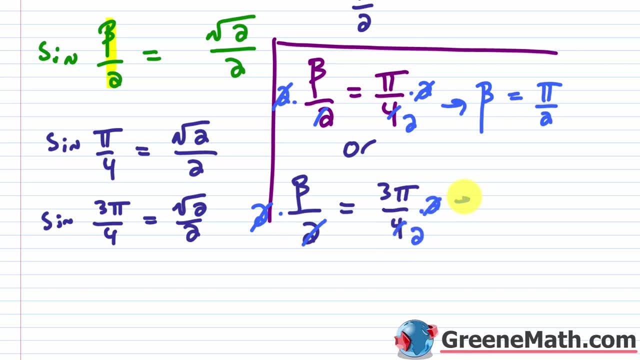 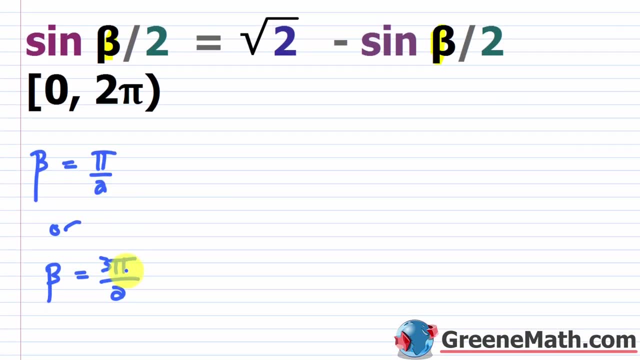 And so this is going to cancel and this is going to give me two here. So we'll say: or beta is equal to my three pi over two. Okay, So these are our two solutions in terms of radians, and they're within our domain or our restrictions. 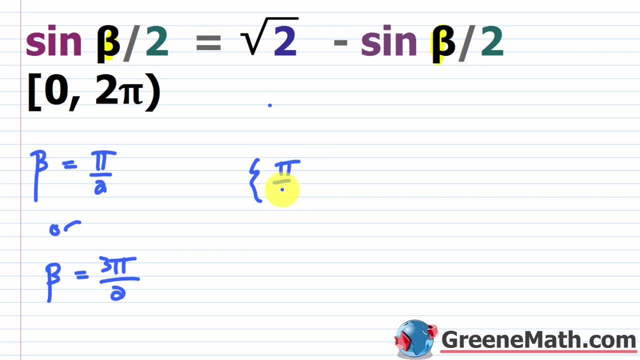 So I'm going to do this in solution set notation. So I'm just going to put pi over two and then comma three, pi over two. Okay, So we're not asked for the general solution here, So we don't need to worry about that. 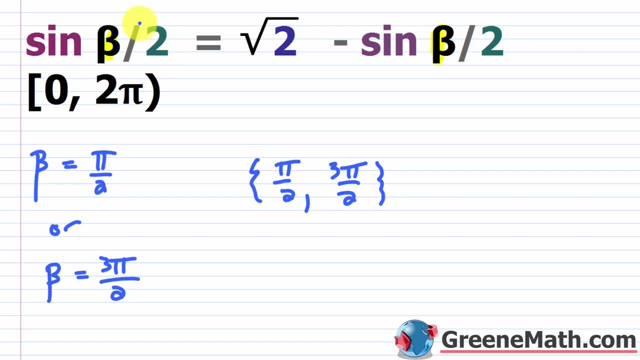 If you were asked for the general solution. Remember, your period here is different because you're dividing by two. So basically, the period here is four pi Okay, Not two pi Okay. So you got to remember that, All right. So one thing I want you to do is pause the video. 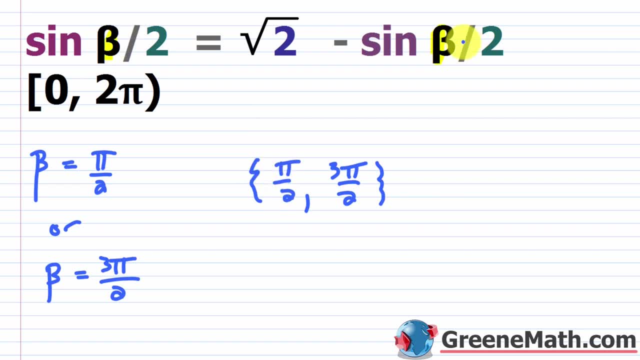 Go ahead and plug pi over two in for beta in each case and verify that, basically, these solutions do work. You can just do one of them. I'm going to just say: trust me that they both work, But just pause the video and see that for yourself. 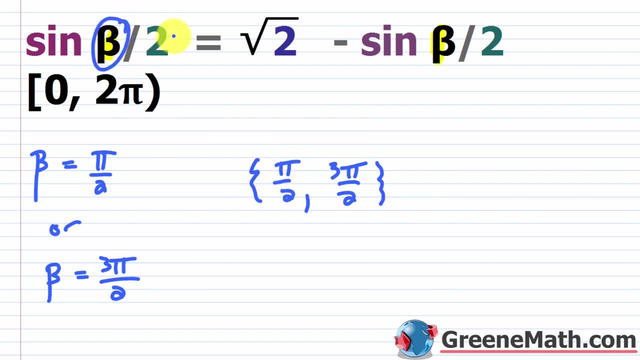 That if you plug in pi over two right here, Okay, So you have pi over two divided by two and right here pi over two divided by two. that basically you would get a true statement: The left side would be equal to the right side. 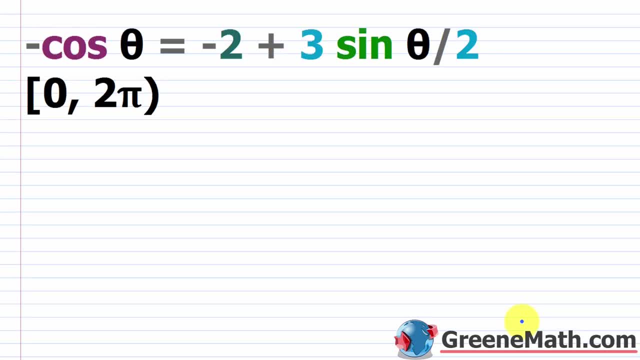 Okay, Let's take a look at another example. So this one is slightly more complex- not more complex, but more tedious, because you do need to use an identity and then there's some squaring involved. So we have the negative cosine of theta is. 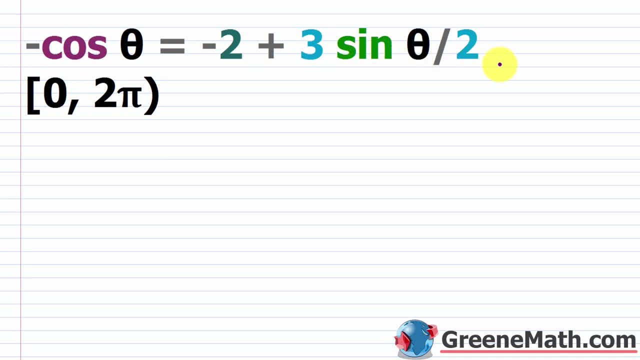 equal to negative two plus three times the sine of theta over two. Again, when you think about these things, if you end up with cosine and then sine, you're going to be thinking about an identity, Right. So if I think about sine of theta over two, if I go back to my handout on the 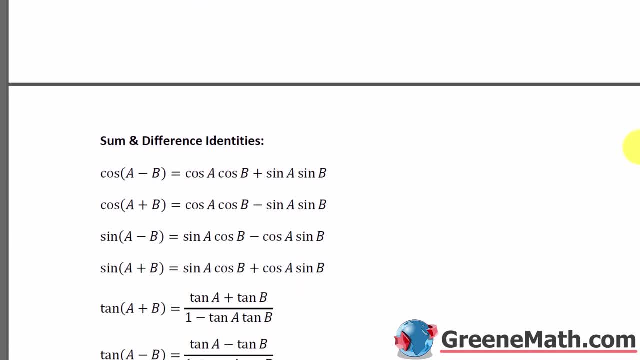 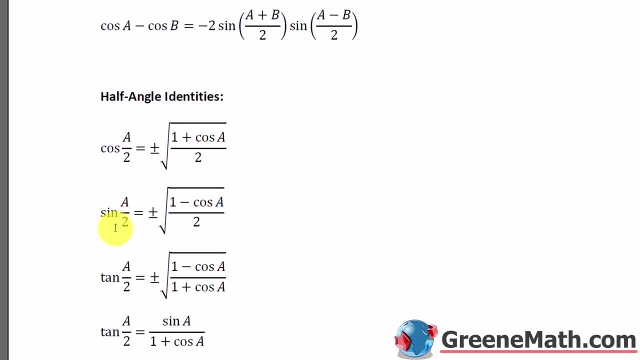 identities and we come down here. let's go all the way down to where we get, to the half angle identities, And was the last one we talked about, So here's the one for sine. So you have sine of a over two. In our case, we're working with theta. 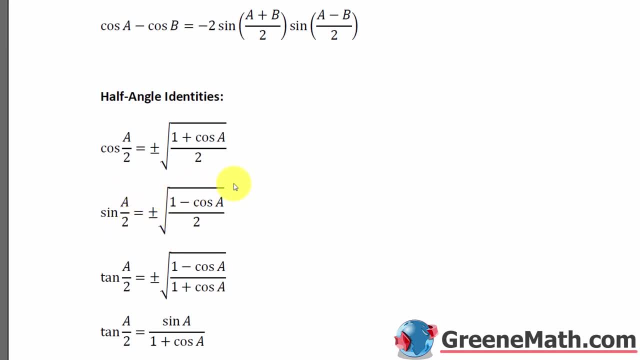 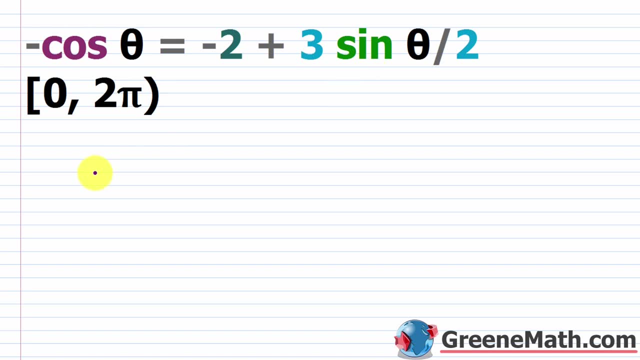 So let's say, sine of theta over two is equal to, plus or minus, your square root of one minus the cosine of theta over two. Okay, So let's go back and let's just make a little replacement. Okay, So I'm going to put the negative of cosine. 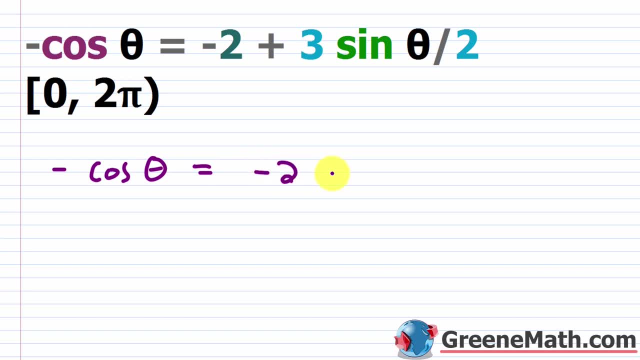 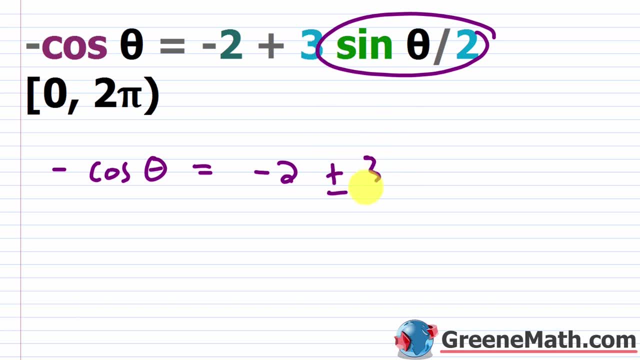 I'm going to put this in front, So I'm going to do plus or minus, like this, and then the three and then times that little guy which was the square root of one minus the cosine of theta, And this was over two. Okay. 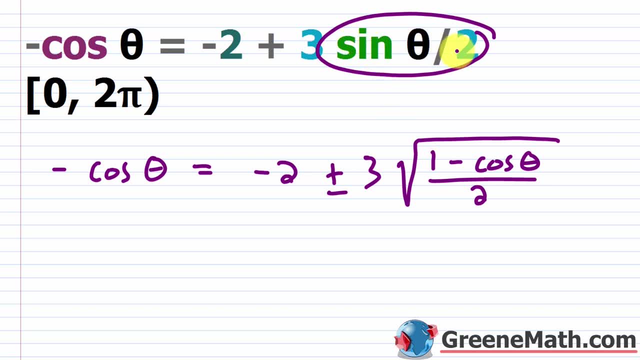 So all I did was I plugged in for sine of theta over two, just using the half angle identity. Okay, It's all I did. Now, what I want to do here: Remember, if you have a radical somewhere, you're going to end up having the square. 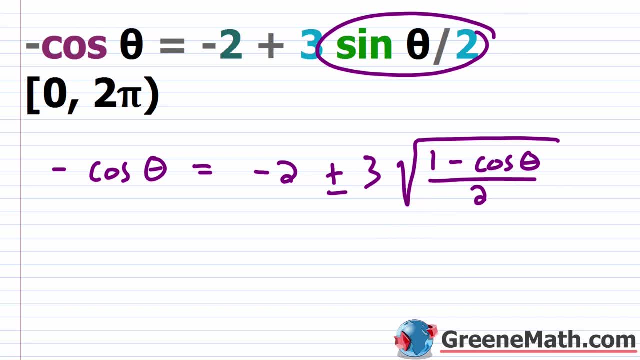 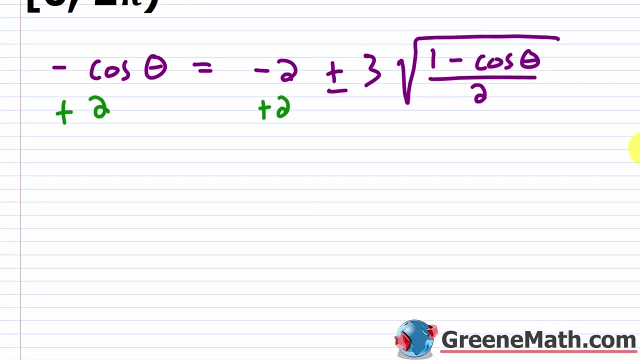 Okay, And in order to do that, you first want to isolate this guy. Okay, So what I would do here is I would first add two to both sides. Okay, And let's scroll down just a little bit. So I'm just going to say that I have two minus the cosine of theta is equal to. 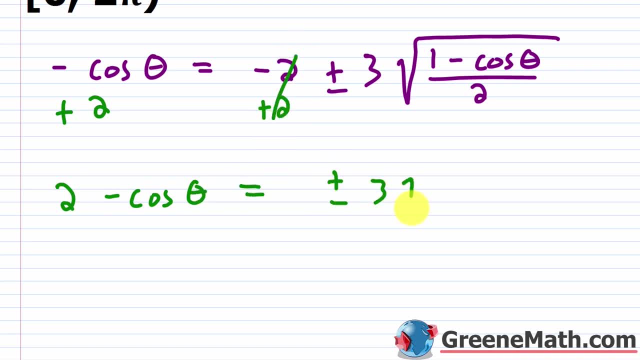 This is canceled over here. So I have plus or minus three times the square root of one, minus cosine of theta over two. Now I can square both sides. Okay, So I can get rid of this radical. So I'm going to square this side. 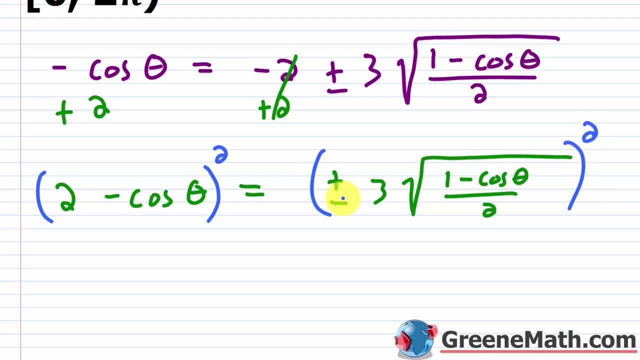 Okay, When you square the plus or minus, you don't have to worry about it, because basically you can think about this as negative one being squared, That's going to be positive one, and a positive you squared, it's still positive. Okay, So you can basically forget about that. 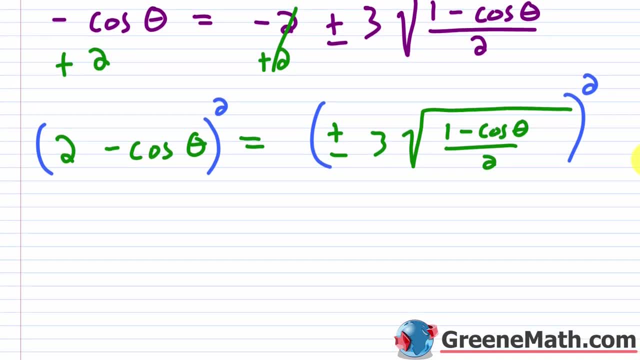 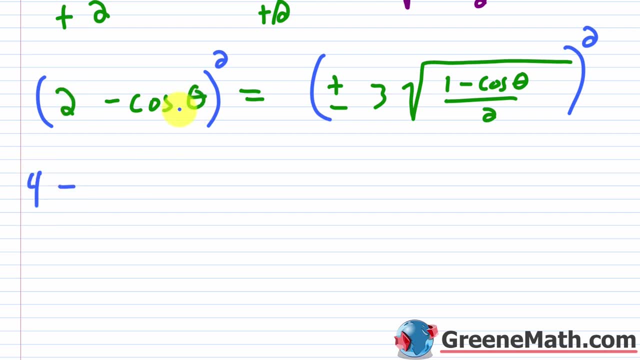 So over here I'm going to use my special product formula and say: it's the first one squared, So two squared is four, and then minus It's two times the first guy, times the second guy. So two times two is four, and then times cosine of theta. 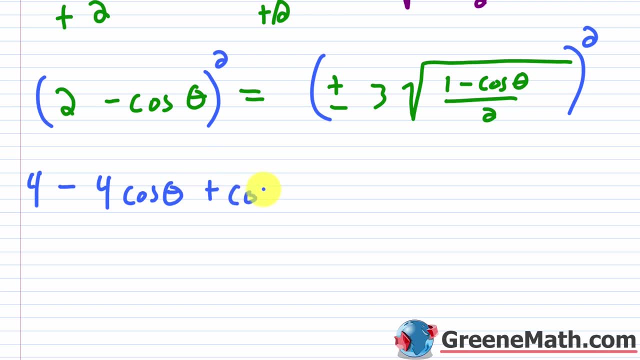 and then plus the last guy squared. So this is just cosine squared theta. Okay, And we'll rearrange this in a moment. I know this is not how we usually write this. We'll put equals again. Don't worry about the plus or minus. that's gone. 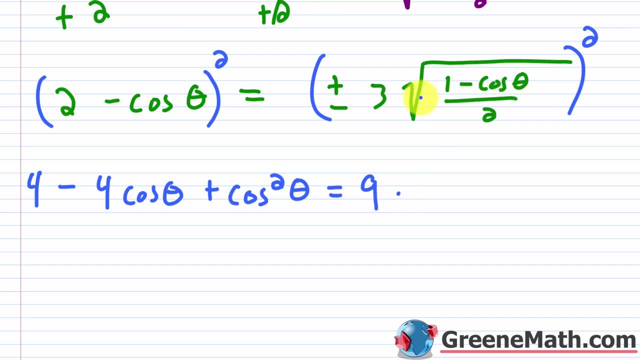 Three squared is going to be nine, and then it's multiplied by this guy right here, Squared. I'm just removing the radical. Okay, So basically you have this one minus the cosine of theta over two. Now be careful here, because nine is multiplying this whole thing. 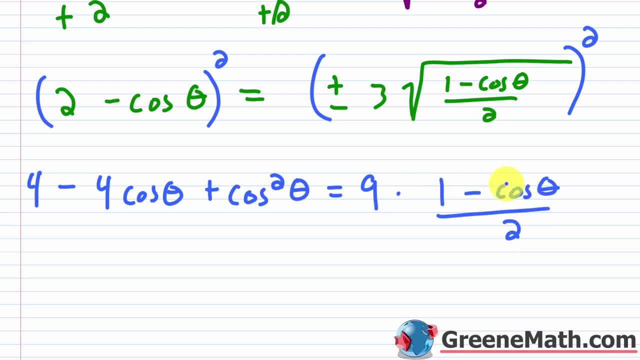 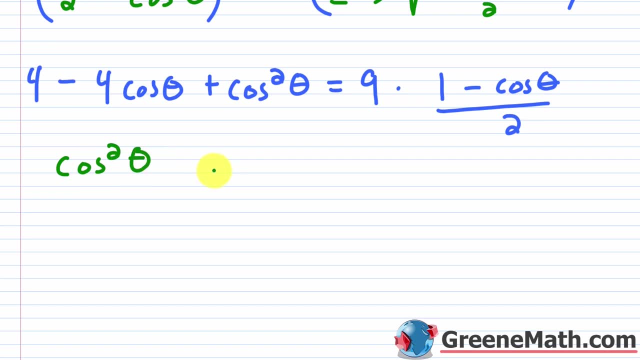 Okay, If you end up distributing this to the numerator, make sure you use parentheses, Very important. What I'm going to do first is rearrange things, So I'm going to put this as cosine squared theta, Okay, Then minus four times cosine of theta and then basically plus four. 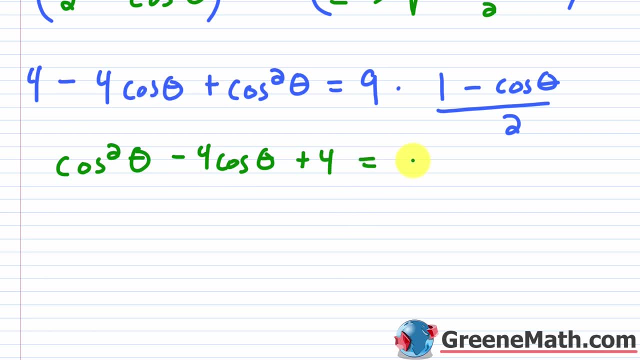 Okay, So I've got all my signs right. I want to make sure on that. And then this equals: let's do nine times one minus cosine of theta, like this: Okay, Because the nine is multiplying the one and also the negative cosine of theta. 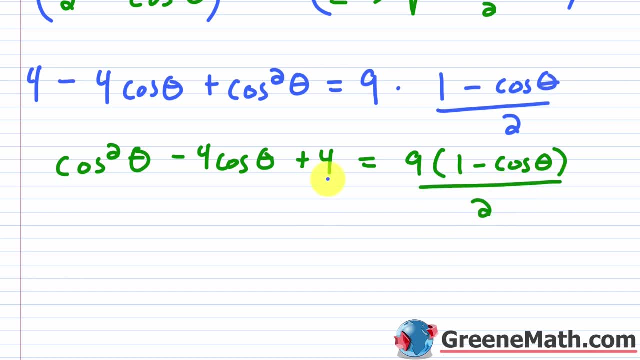 Then this is over two. Okay, So now what I'm going to do is I'm going to multiply both sides by two so that I can clear this denominator. Okay, So basically, this comes here and cancels here, And here I'm just going to put a two. 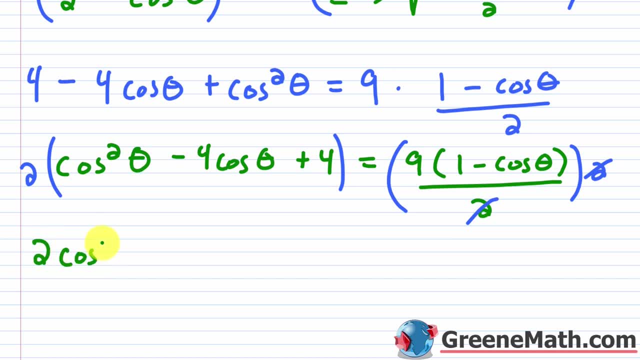 Okay, Being multiplied by everything there, So you'd have two times the cosine squared theta, And then I would basically have minus eight times the cosine of theta, And then plus I would have eight, and this equals the two is canceled. So just let's go and distribute this. 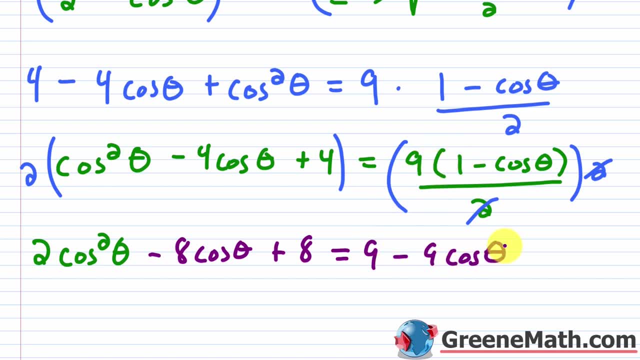 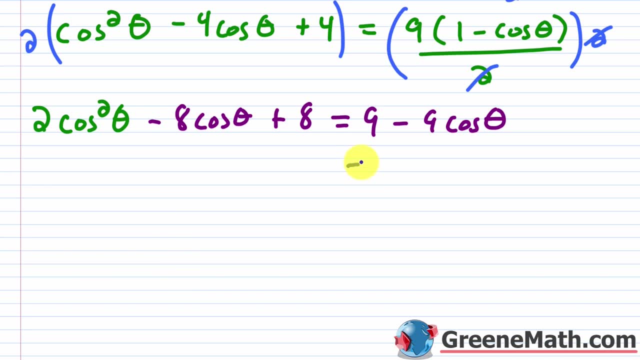 So nine minus nine times the cosine of theta. Okay, So so far so good. Let's scroll down just a little bit more, Okay? So what I want to do here is basically subtract nine away from each side of the equation and also add nine times the cosine. 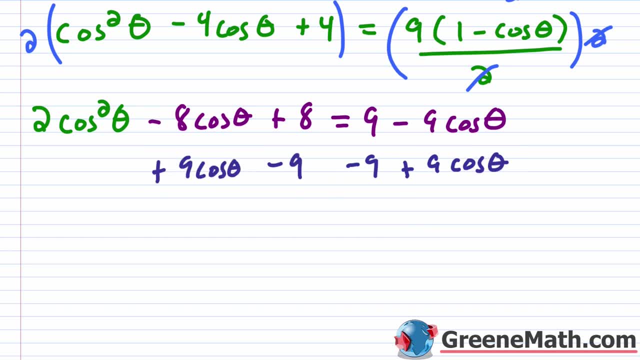 of theta to each side of the equation, Okay, So basically, what this is going to do is give me a zero on the right. Okay, You can see where I'm going with this. I'm going to end up factoring and using the zero product property. 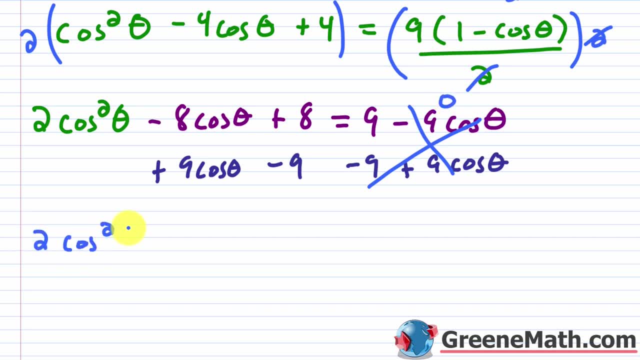 So on the left I have my two times the cosine squared theta And then basically I have negative eight cosine of theta plus nine cosine of theta. So this is going to be plus cosine of theta, or you could say plus one times the cosine of theta. whatever you want to do there. 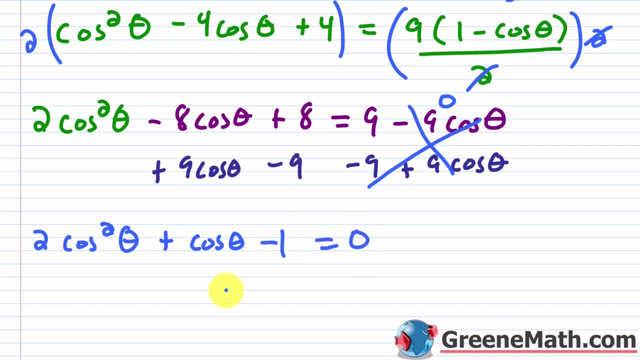 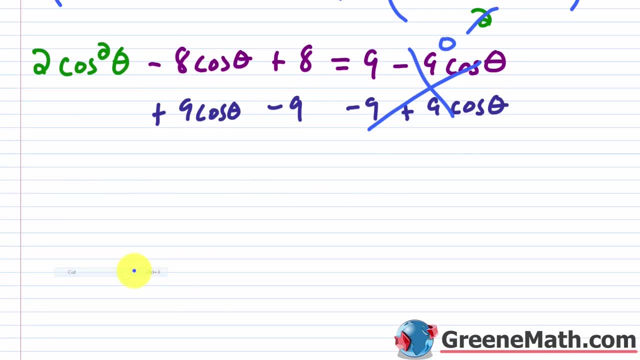 And then, basically, eight minus nine is negative one, and this equals zero. Okay, So the idea here is that, of course, if you wanted to, you could use the quadratic formula, but we have something that is factorable, So let me go ahead and cut this away. put that in there. 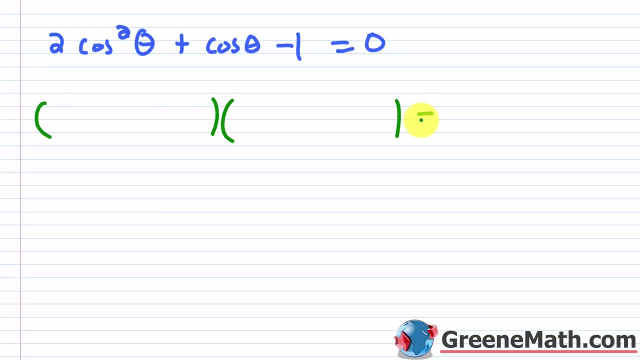 So I'm just going to factor the left side here Again, if you have trouble factoring this- I see a lot of students having trouble write it as two u squared plus u minus one equals zero. You can factor that, no problem, right. 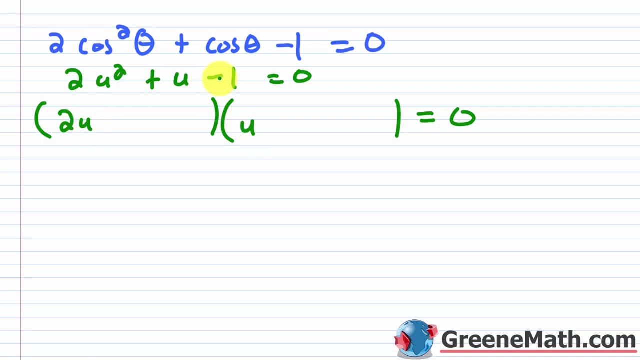 You think about this as two u and u, And then the last guy here is a negative one, right? So that tells me I need mixed signs here. This guy is going to be positive, So what I want to do is put a plus one here and a minus one here, right? 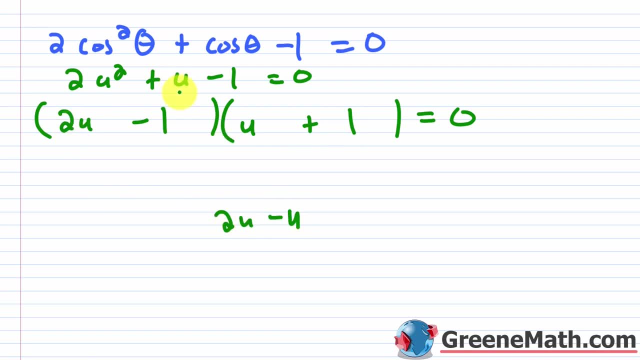 Because the outer would be two u and the inner would be minus u, So that would give me the correct plus u there. Okay, Now, once you've factored it like this, you just put your cosine of theta in for u. Okay. So let's come back in here. 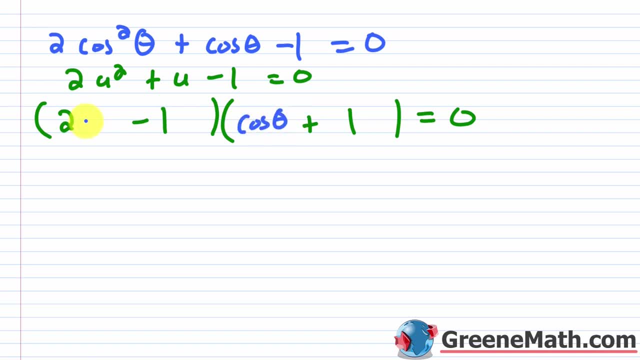 I'll place this with cosine of theta and your roadblock is gone. Okay, So two times cosine of theta there, Okay, So a little trick for you. Now I'm going to set each one of these equal to zero and solve. Let me just get rid of this. We don't need this anymore. 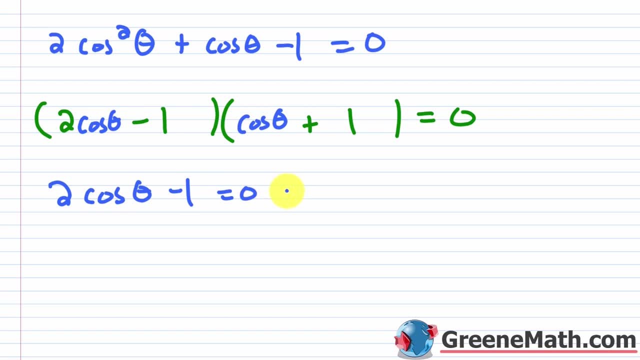 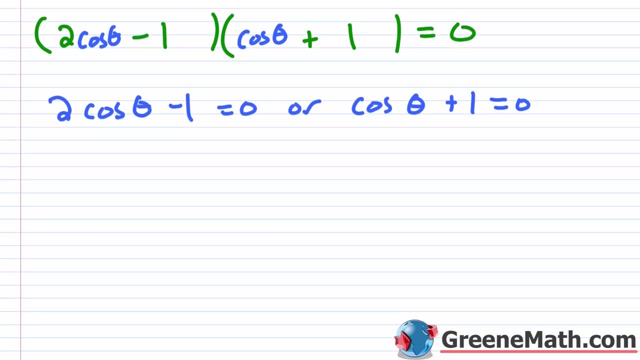 So I'll say two times the cosine of theta minus one equals zero. Or I'll say the cosine of theta plus one equals zero. Let me scroll down and get a little room going here, So basically I'm going to add one to both sides. 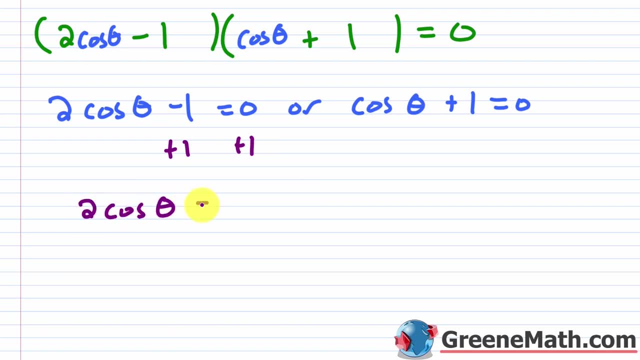 and this is going to give me two times the cosine of theta is equal to one. Okay, I'm going to now divide both sides by two and I get cosine of theta is equal to one half. Okay, Over here let me go ahead and put: or. I'll put or. 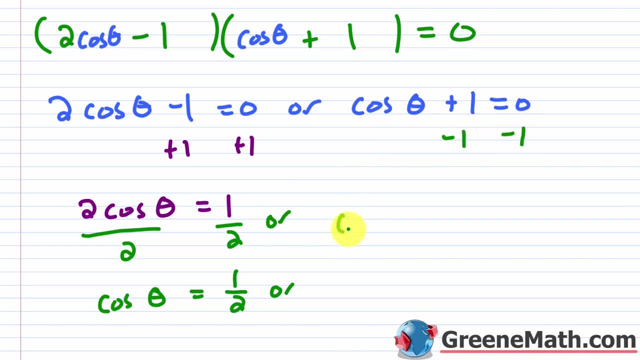 And then over here I'm just going to say: minus one, minus one, So the cosine of theta is equal to negative one, And I guess I don't really need another one here. So let's put this over here. Well, I guess I could write it in here. 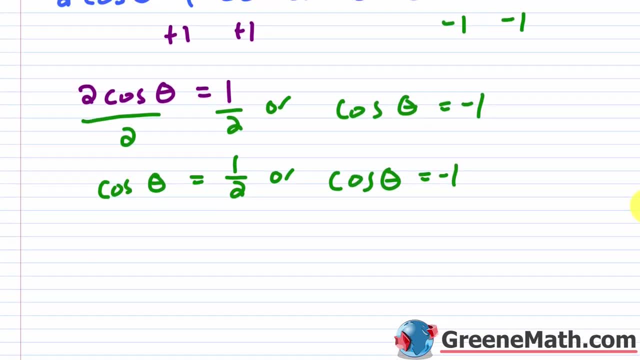 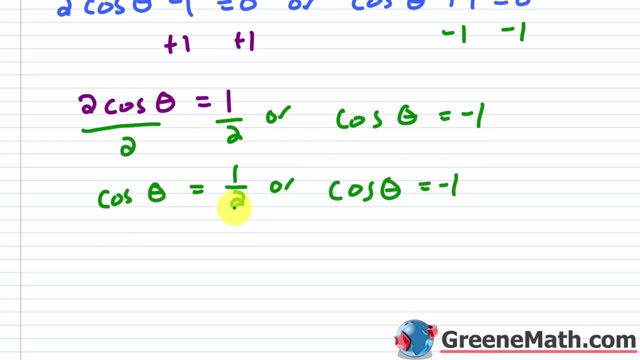 So cosine of theta equals negative one. Okay, So you see what we're doing here. We basically have to solve this guy and then this guy. So where's cosine going to be equal to a half? Remember, cosine is positive in quadrants one and four. 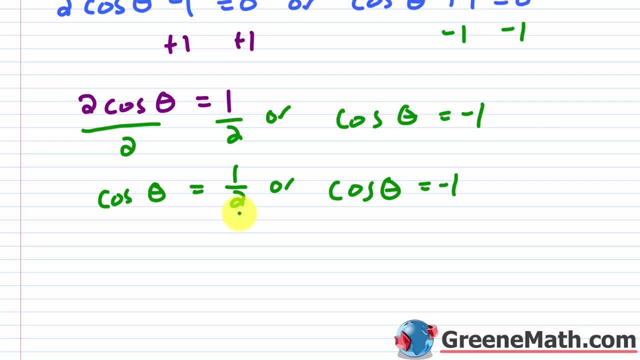 And we know that cosine of 60 degrees, okay, is a half. So basically you would want a 60 degree reference angle in quadrant four, So that would be 300 degrees, right? So you'd want 60 degrees And then 300 degrees. 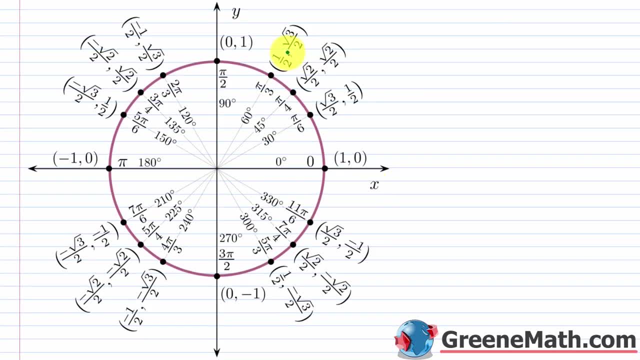 Again, if you're still looking at your unit circle, it's no big deal, right? This is a half here. So you see it's 60 degrees, or pi over three in terms of radians, And then over here you'd be in quadrant four. 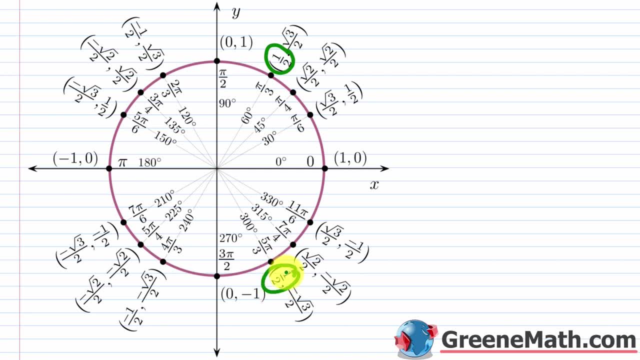 So you have a half here, 300 degrees, or five pi over three in terms of radians, Okay. So again, if you need to use the unit circle, keep doing it, You will memorize it eventually. Now, while we're down here, 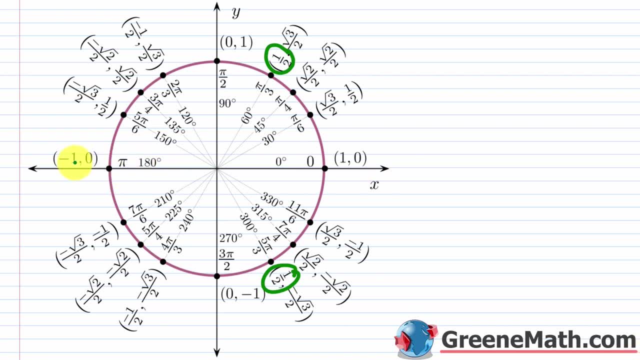 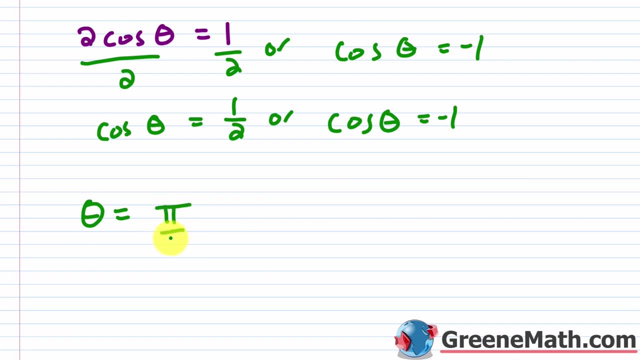 I might as well note that basically, pi cosine of pi is going to give you negative one. So let's go back up and let me erase the degrees and let me say that theta here would be equal to your pi over three, and then it would be five pi over three. 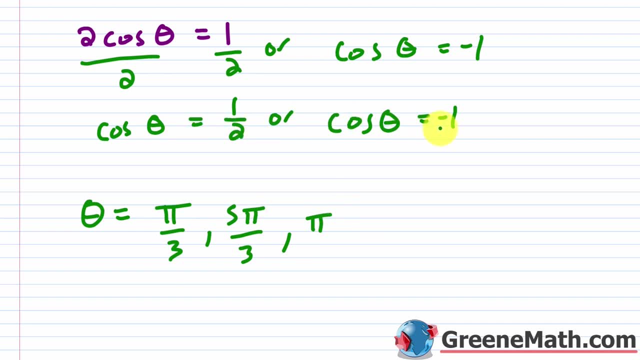 And then it would also be pi right. So this covers these solutions from these guys. Now, in order to make the video a little bit shorter, a little bit more concise, I'm not going to check these solutions when you square both sides of an equation. 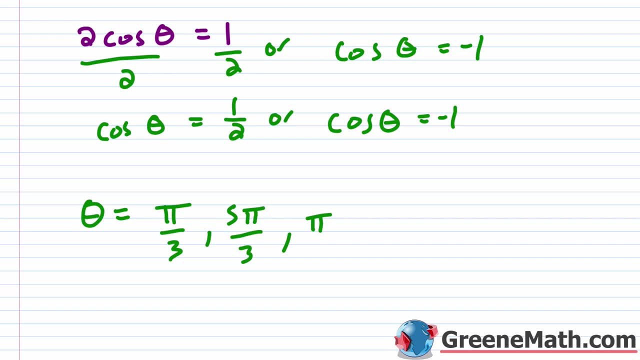 We know from basic algebra that there's a possibility of extraneous solutions, right Solutions that won't work in the original equation. I have already checked this. I know that these guys are going to work. I can say that solution set here is pi over 3, okay, And then I'll say pi, and then I'll say 5, pi over 3, like. 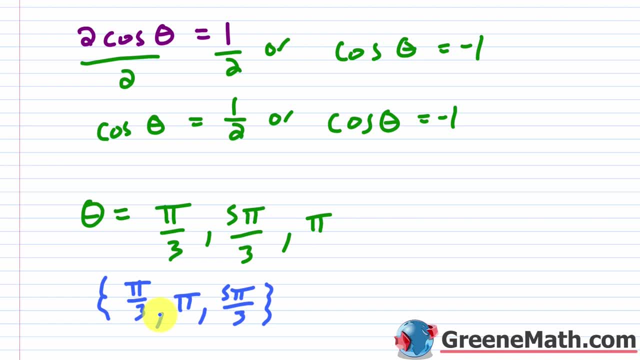 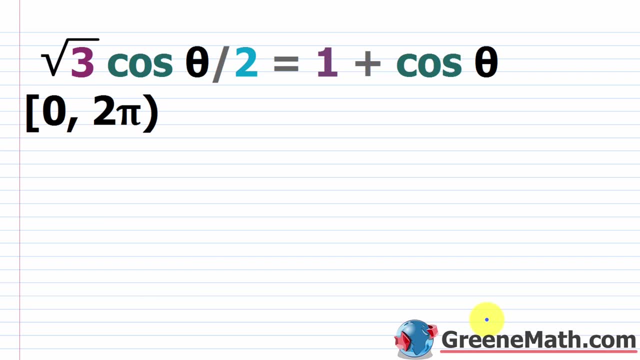 this okay, So these solutions do work in the original equation And the next example. we'll see where it doesn't okay, So let's go to that now. All right, Let's look at another example here. So we have the square root of 3 times the cosine of theta over 2 is equal to 1, plus the cosine of. 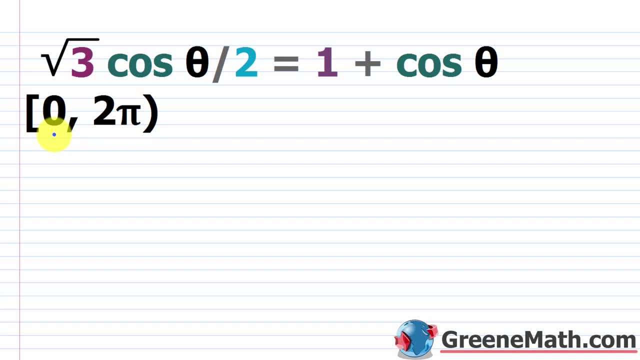 theta. okay, Again, same interval from 0 to 2 pi 0 is included Again. if you see something like this: you have cosine of this and cosine of this. Well, you can go ahead and use your identity. So. 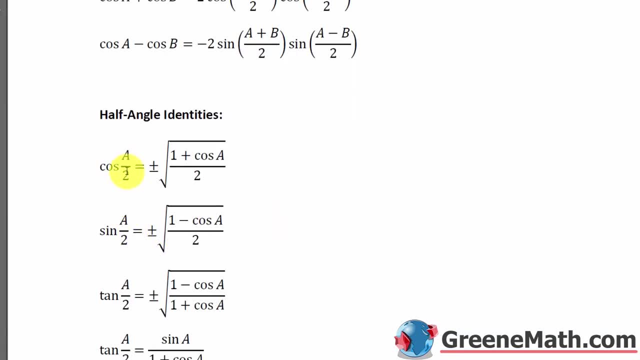 we come back here Now. cosine of, in this case would be theta. theta over 2, is plus or minus the square root of 1 plus the cosine of theta over 2.. So let's just make a little substitution here. 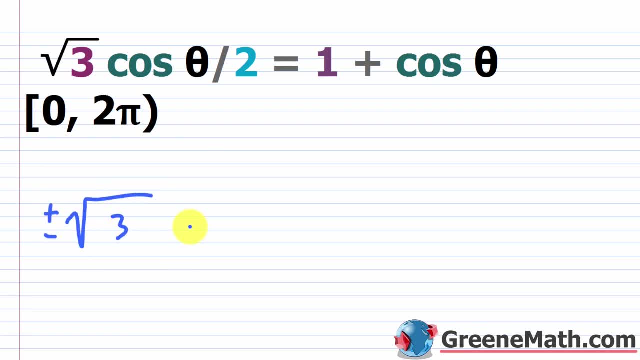 I'll say the square root of 3, okay, And I'll put the plus or minus out in front of here. then times my square root of 1.. In this case it's plus the cosine of theta, Remember if it's. 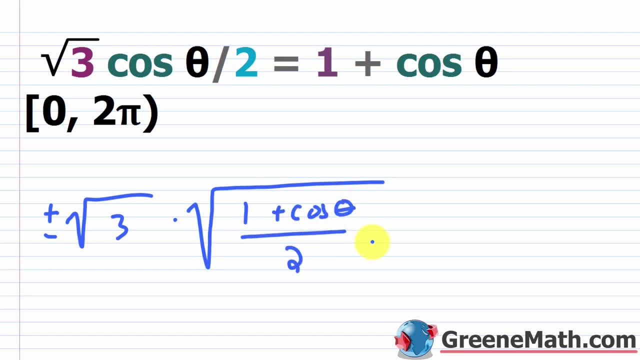 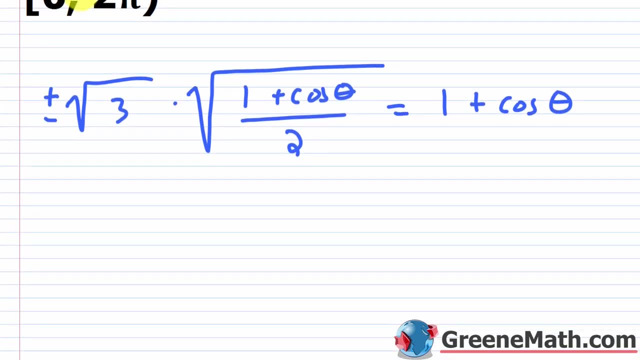 sine, then it's minus. If it's cosine, it's plus, Then this is over 2. And this equals your 1 plus your cosine of theta. okay, So again, all I need to do here is just square both sides. So let's square this side and let's square this side. okay, And over here. 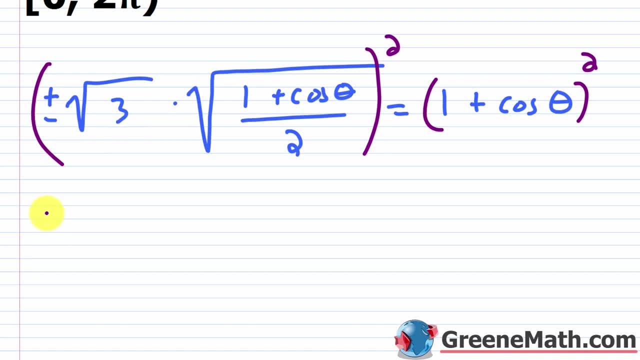 the plus and minus. forget about it, it's gone. Square root of 3 squared is 3.. This guy, if I square it, I'm basically going to end up with the radicand. So this is 1 plus the cosine of theta. 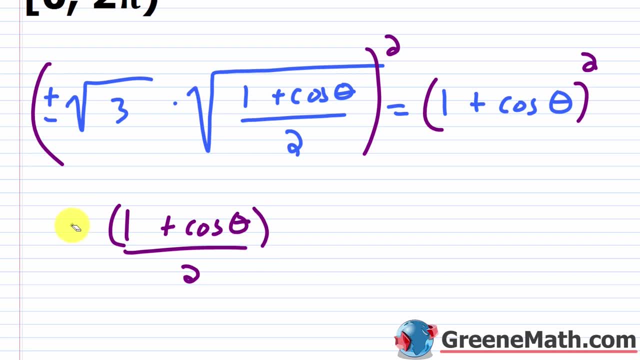 over 2.. And to speed this up, let me just wrap this in parentheses and put this like this: And let's put equals over here. I'm going to flip these, I'm just going to put the cosine of theta plus 1,. 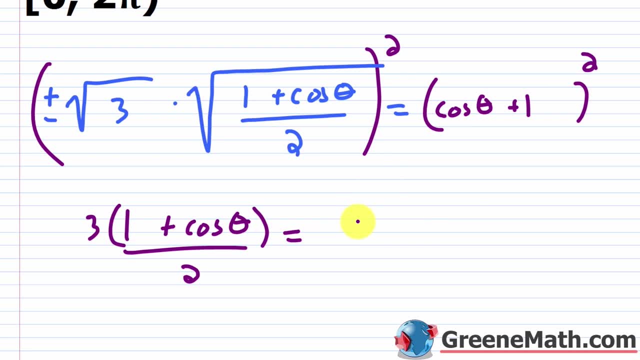 so it makes it easier. So cosine of theta plus 1, like this. So this would be the cosine squared theta first guy squared plus 2 times the first guy times the second guy. So it's basically just 2 times cosine of theta and then plus the last guy squared, so that would be 1, okay. 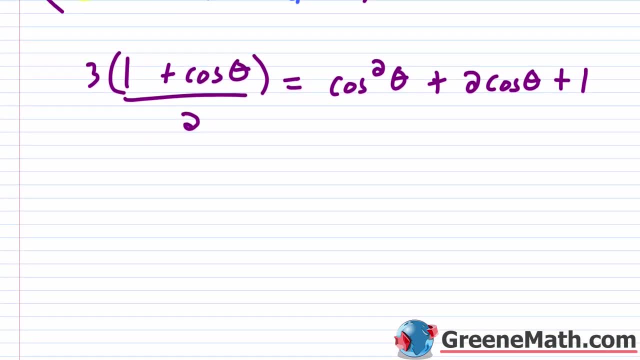 So, over here now all we need to do is basically multiply everything by 2, right, So this would cancel. Let me show this visibly And let's go over here and do this. So now I have 3 times 1,, which is 3,, plus 3 times the cosine of theta, And this equals 2 times the cosine squared theta. 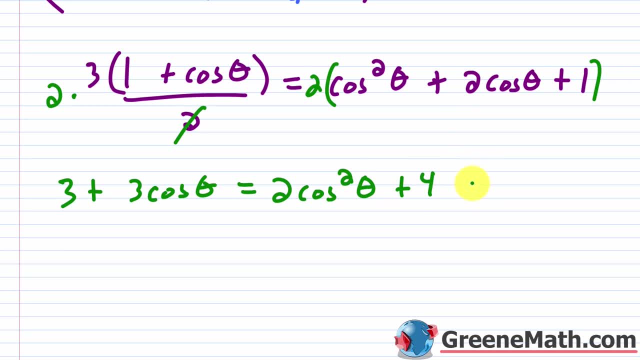 plus you'd have 4 cosine, and I messed that up- So cosine of theta. and then plus 2 times 1 is 2.. So from here, because I have a squared term, I want to think about either factoring or using. 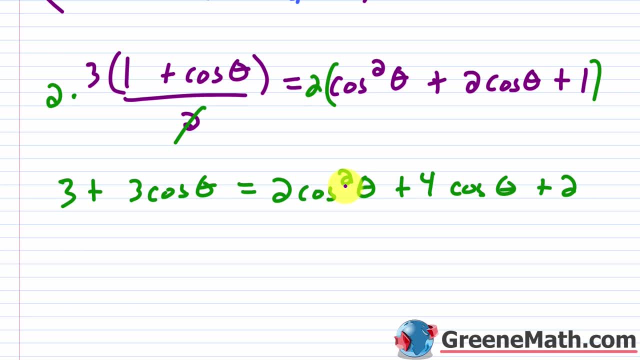 the quadratic formula. This one's going to be factorable, so we'll be safe there. Basically, let's move everything to the left, because that's where I like it, So let's subtract 2.. So, basically, this is going to be: 1. Let's go ahead and subtract. 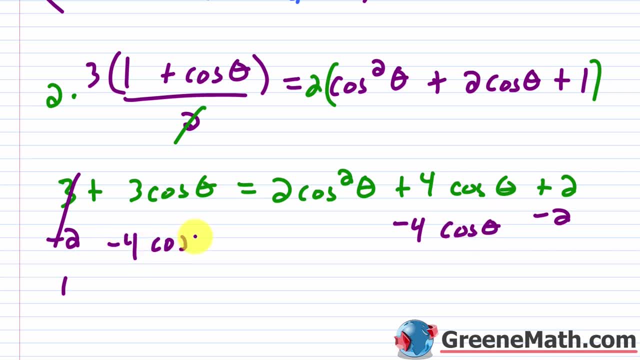 4 times the cosine of theta. So minus 4 times the cosine of theta, So this is going to be negative cosine of theta. And then let's subtract 2 times cosine squared theta. So I'm running out of room over here, so let's just kind of put this over here. So minus 2 times cosine squared of. 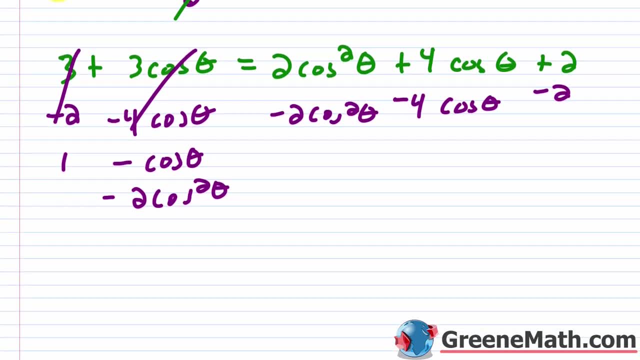 theta. I know this is kind of getting a little messy, but let's just write it neatly now. So we'll put this out in front. We'll put negative 2 times cosine squared theta, And then we'll put minus cosine of theta, Then we'll put plus 1. And of course everything's. 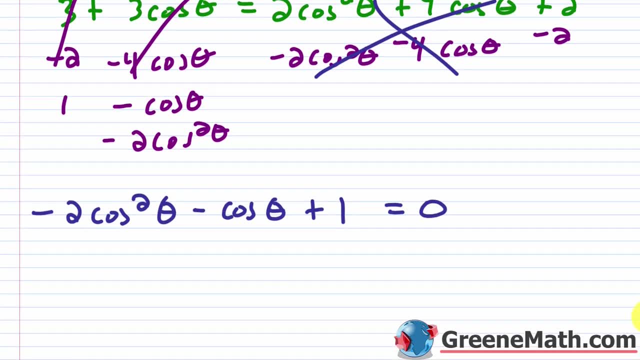 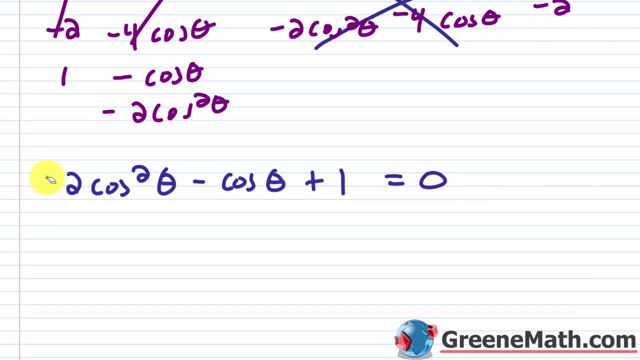 gone from over here. So this equals 0.. If you want for factoring- a lot of people do not like to factor with a leading coefficient, that's negative- You can multiply everything by negative 1.. So this becomes positive, This becomes positive, This becomes negative And it has no effect on 0.. 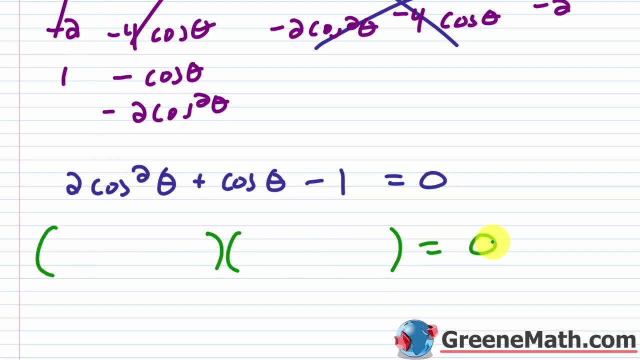 So, basically, if I want to factor this again, you can use that trick with U if you want. I don't really need to do it. So I'm just going to put 2 times cosine of theta and cosine of theta, because this times this would give me this. Now the final guy is negative 1.. 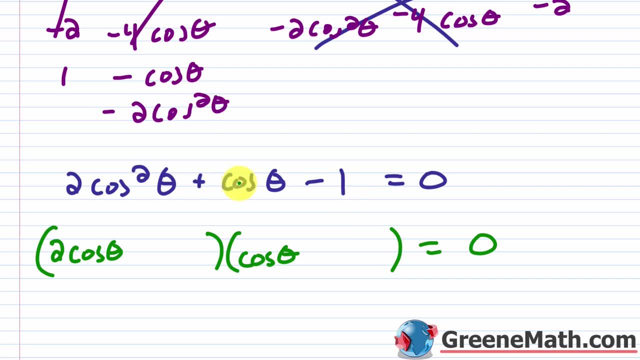 So that can only come from positive 1 times negative 1.. We know that this guy right here is positive, So that means I want to put plus 1 here and minus 1 here, right, Because the outer will be 2 times cosine of theta, The inner will be minus cosine. 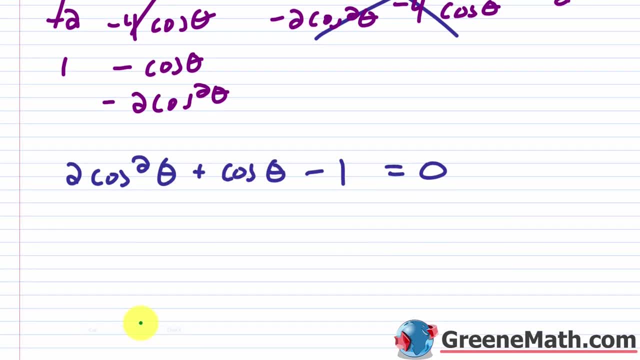 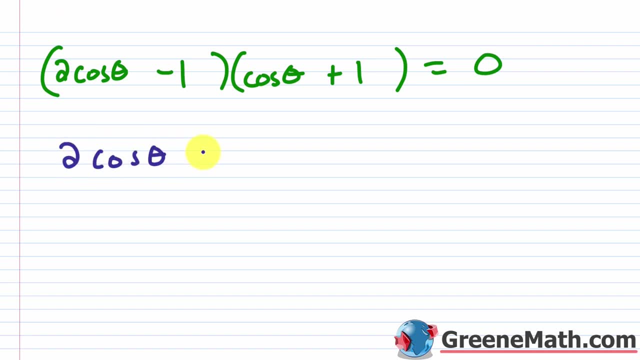 of theta. So that will combine to give you this okay. So let's go ahead and copy this and paste this in another sheet And again I'm just going to use my zero product property. I'm going to say 2 times the cosine of theta minus 1 equals 0, or the cosine of theta plus 1 equals 0. 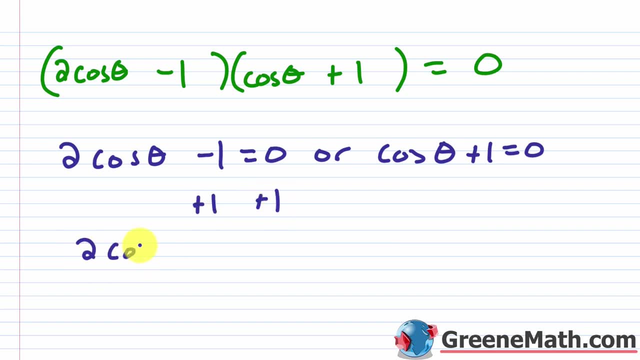 So I'm going to add 1 to both sides over here And I'll have 2 times. the cosine of theta is equal to 1.. Divide both sides by 2. And again we get this cosine of theta is equal to a half. 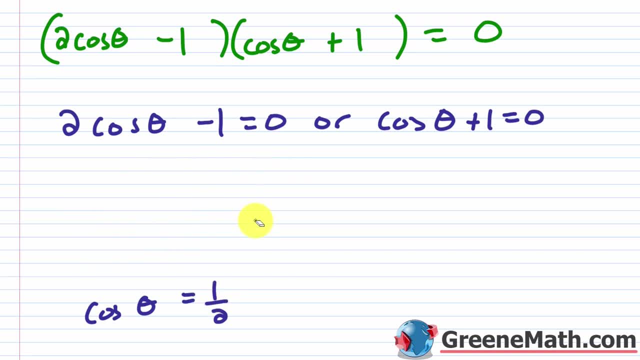 So we already know that that's going to occur basically at 60 degrees right, Or a reference angle of 60 degrees in quadrant 4, which is 300 degrees. Let me just drag this up here. We'll say that theta here is 5 pi over 3.. Or actually, let's do this first, So we'll do. 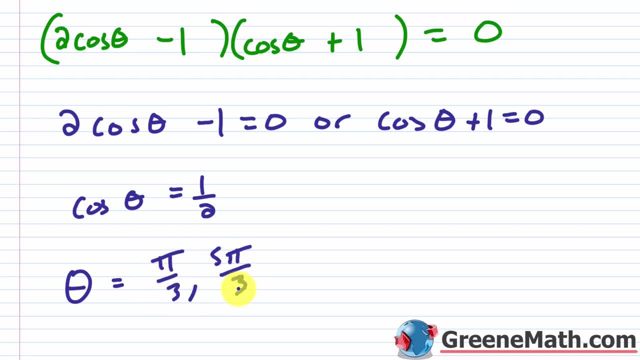 pi over 3, or then 5 pi over 3.. So again, this guy right here is your 60 degrees. This guy right here is going to be your 300 degrees. okay, So then, or okay, And I'll just: 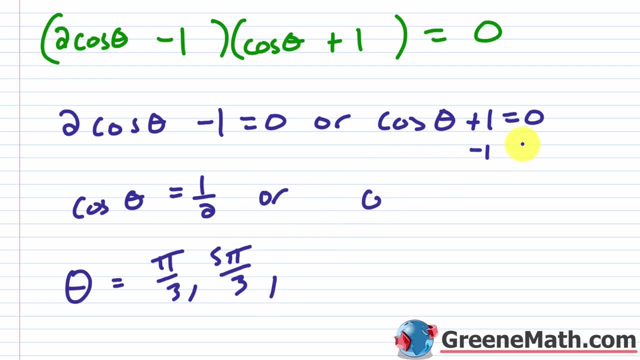 put a comma here For this one. it's really simple. I just go minus 1 here, minus 1 here. So we have the cosine of theta is equal to negative 1.. We already know this is going to be pi, okay. 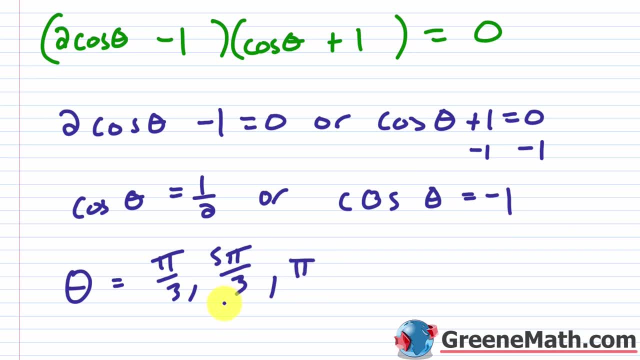 So we've seen this before. So this is exactly the same solution that we got in the last section or the last example, But basically now you're going to see that one of them is not going to work, So let's actually erase all of this. We know it's a pain to check solutions, but it's. 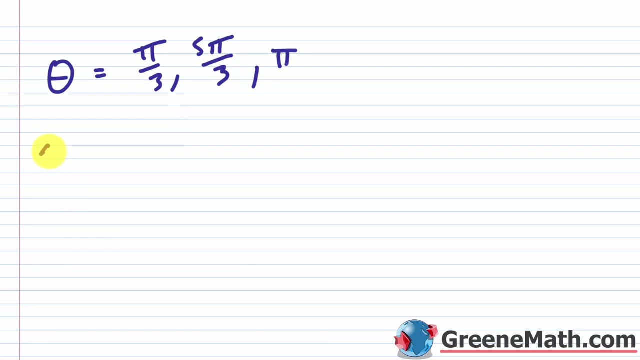 absolutely necessary in this case. So my original equation is the square root of 3 multiplied by the cosine of theta over 2, okay, And then basically you have is equal to 1 plus the cosine of theta. So what do I have here? to start, Let's go square root of 3 times. 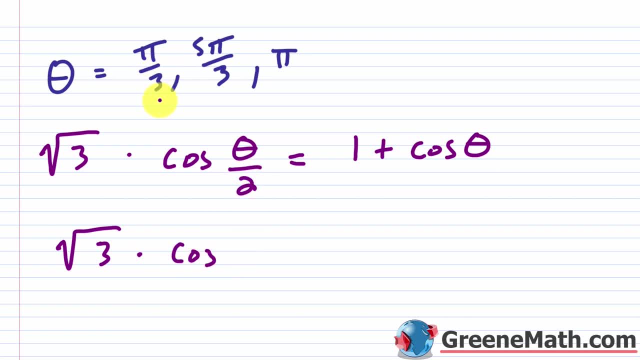 you would have the cosine of: basically, you would have pi over 3 divided by 2.. So it's like multiplying by half. So it's the cosine of pi over 6.. And the cosine of pi over 6, remember, pi over 6. 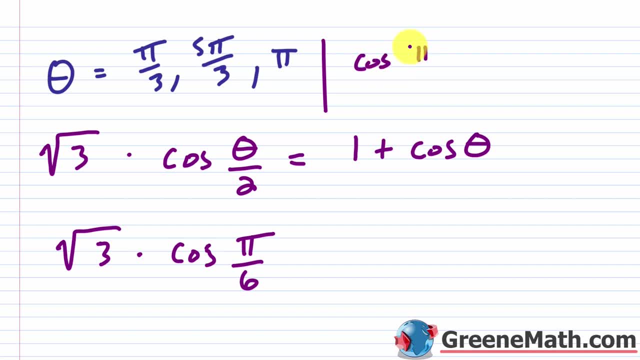 is square root of 3 over 2.. So let me just write this over here for reference. So cosine of pi over 6 is square root of 3 over 2, okay. So let me erase this and I'm going to put square root of 3. 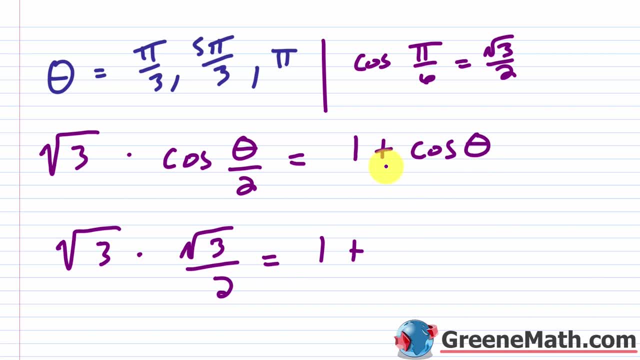 over 2. This equals 1 plus the cosine of theta. In this case we're working with our pi over 3.. Let me write this in: So the cosine of pi over 3.. And we already know that this is 60 degrees here. So this: 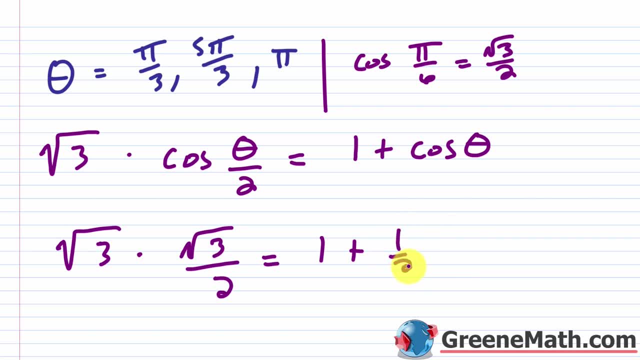 would be 1 half. okay. So what is 1 plus 1 half? Most of you know this would be 2 over 2 here. So 2 over 2 would be 3 over 2, or basically 3 halves. Now, if I do square root of 3 times square root of: 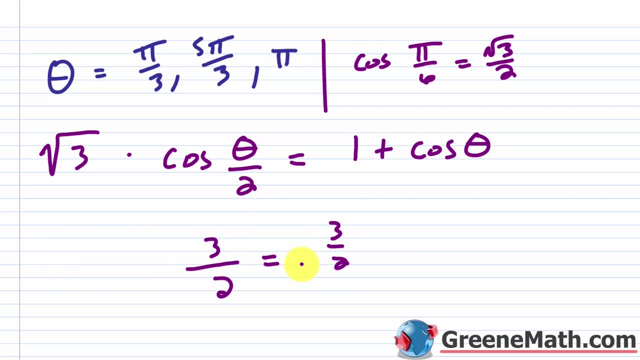 3, that is 3, okay. So this does give me 3 halves. So the first solution is valid. So this one you can put a big fat check, okay. The next one you're going to see a problem with. So let's go ahead and 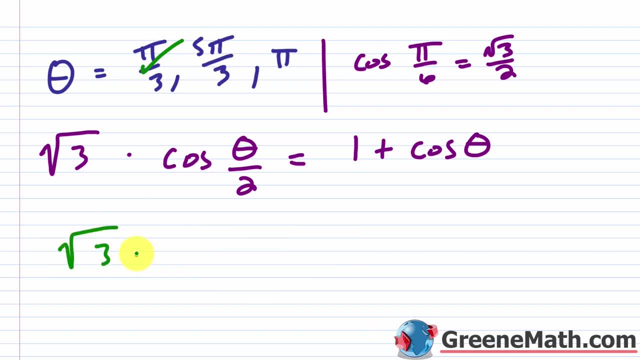 erase this and try again. So we have the square root of 3 times. I'm putting 5 pi over 3 in here. Remember, if I do 5 pi over 3, let me erase this. we're not going to need this anymore. So if I do, 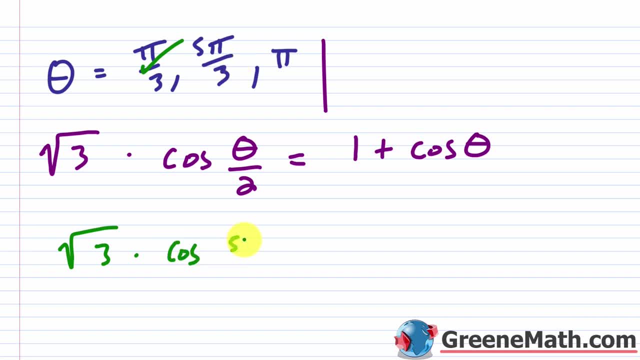 square root of 3 times square root of 3, and then divide it by 2, it's like having cosine of 5 pi over 6.. Now 5 pi over 6 is 150 degrees, so that has a 30 degree reference angle And it's in. 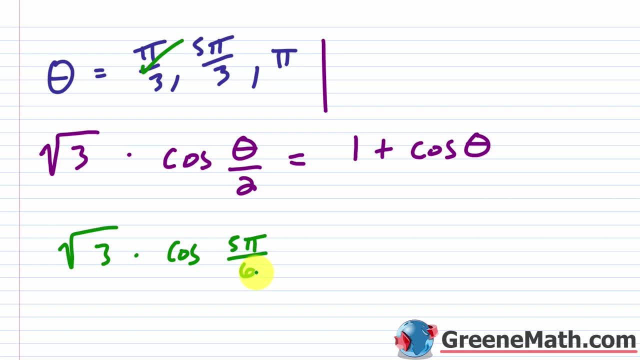 quadrant 2,. so it would be the negative of the square root of 3 over 2,. okay, So this is the negative of the square root of 3 over 2,. okay, Over here I have 1 plus the cosine of 5 pi over. 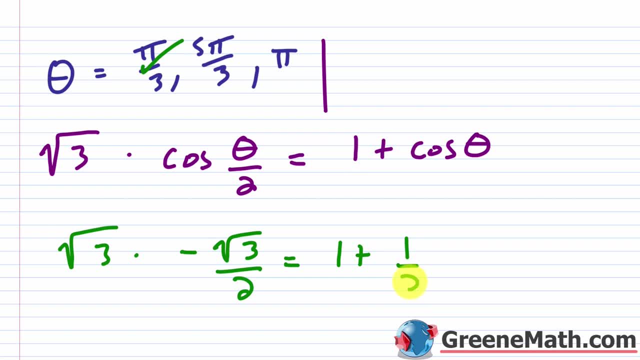 3. And we already know this is going to be a half right, So we know this is a half. this ends up here And you can see this is not going to work out because of the sign right Square root of 3 times. 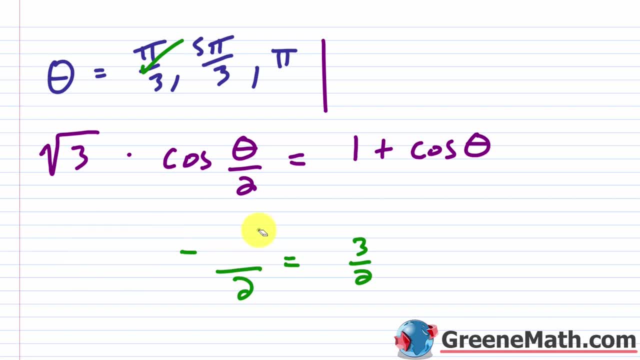 square root of 3 is still 3, but now it's going to be basically negative. of 3 halves equals 3 halves, so this is false right. This does not work. So this is what I mean by checking the solutions. 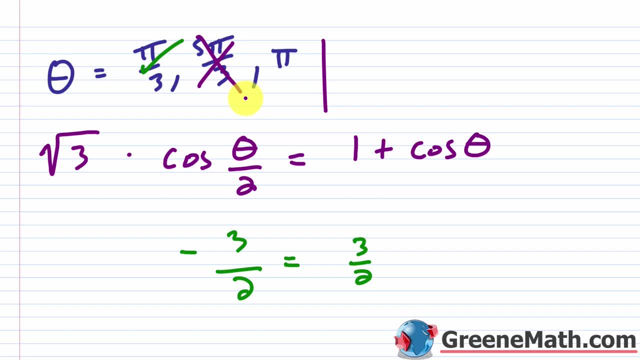 If you don't check them. there's a chance. it's not going to happen every time, but there's a chance that you report a wrong answer. okay, Something that doesn't work in the original equation. Now this last one's going to work If I put a pi over 2 in here. remember pi over 2 is 90 degrees and 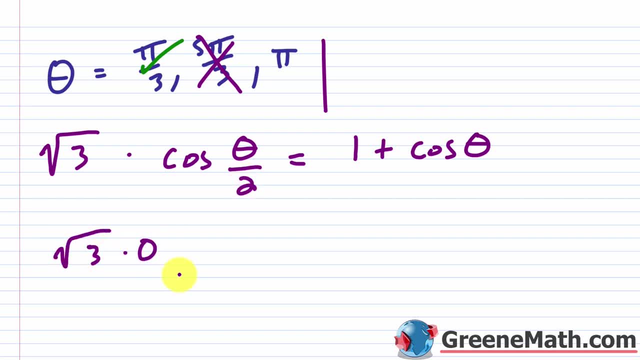 pi over 2 is 0, right. So if I did square root of 3 times 0, well, that's 0, right. So you can basically say this is 0 over here, And then on this part I have 1 plus the cosine of pi. 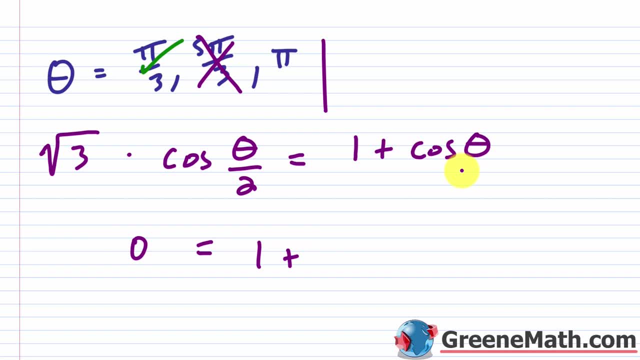 and the cosine of pi, or the cosine of 180 degrees, is going to be negative 1.. So what is 1 plus negative 1?? That's going to be 0. So you get 0 equals 0, so this one checks out as well. okay, So let's go ahead and erase this and we can finally write. 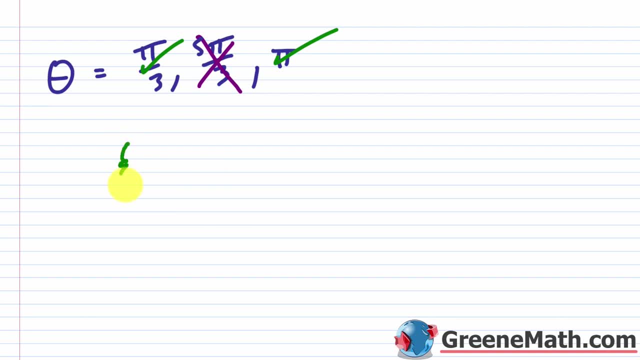 our solution set. I know this is super tedious, but it's just something you have to do. So we end up with pi over 3, okay, And then we end up with pi. These are the only two solutions in the interval we're given from 0 degrees, or from actually 0 in terms of radians out, to 2 pi. 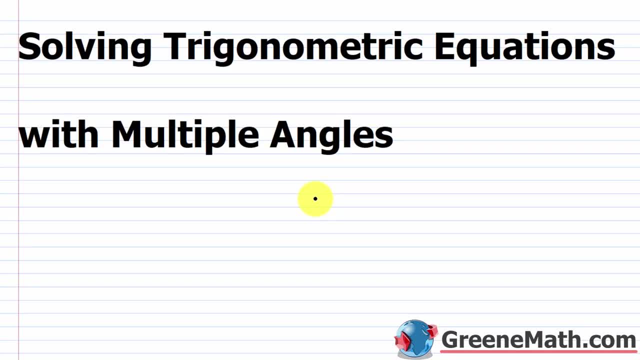 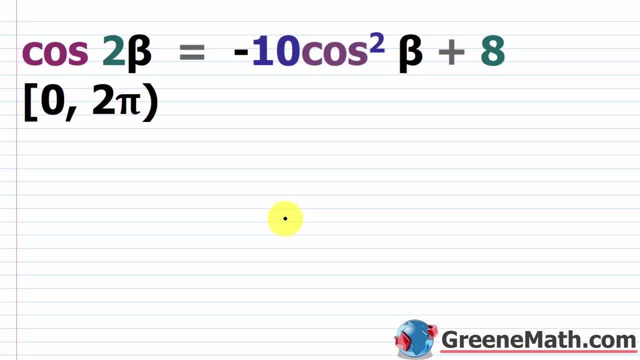 in terms of radians. So 0 is included. 2 pi is not In this lesson. we want to talk about solving trigonometric equations with multiple angles. All right, let's take a look at the first problem. So here we have. the cosine of 2. beta is equal to negative, 10 cosine squared beta plus 8.. 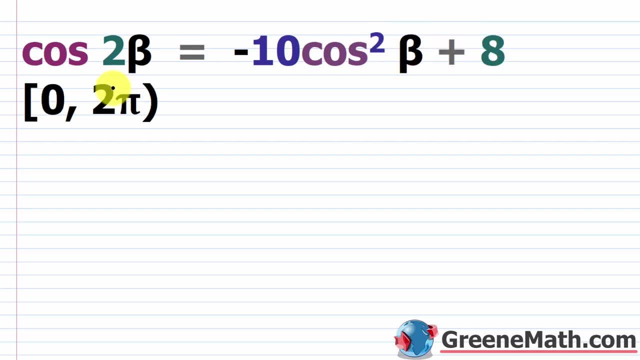 Now we just want to solve this from 0 to 2 pi, where 0 is included and 2 pi is excluded. Now, when you look at this, if I'm trying to get, cosine of beta equals some number, here you have cosine of. 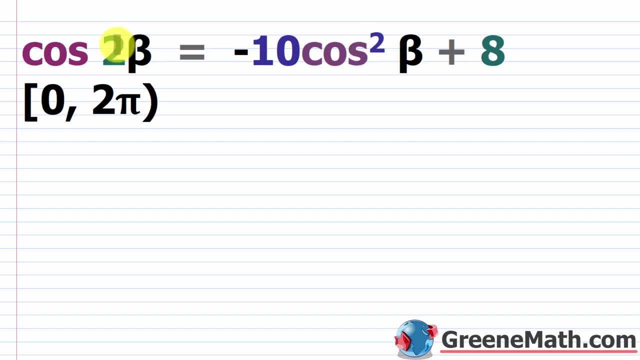 2 beta. here you have cosine squared beta, So this one right here is going to be the immediate problem for us, because you want to write this in terms of the cosine of beta again equals some number in the end. So what you would want to do is use a little identity to plug in for this guy and you want to write this down. So what you want to do is use a little identity to plug in for this guy and you want to write this down. So what you want to do is use a little identity to plug in for this guy. 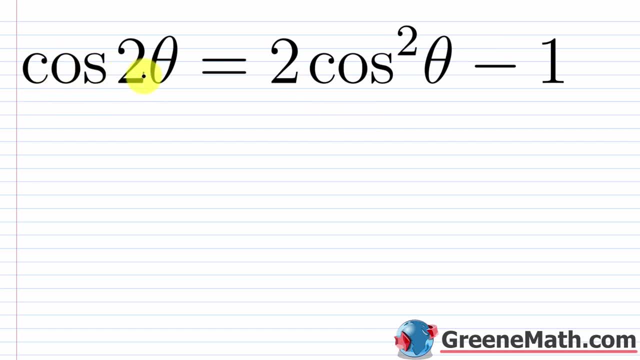 this is the one I'm going to work with. If you have cosine of 2 theta or 2 beta- whatever you're working with- you have three different formulas you can choose from. I'm going to work with this one. So what I'm going to do is say the cosine of 2 beta is equal to 2 cosine squared beta minus 1.. 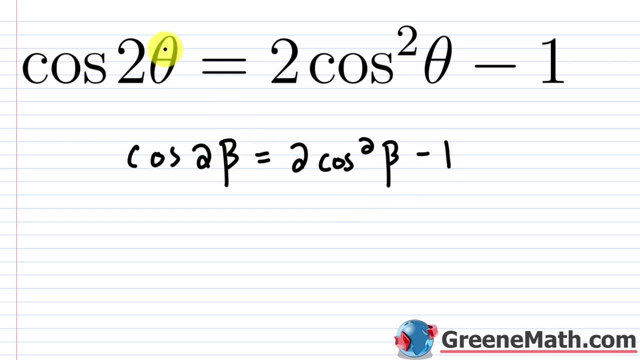 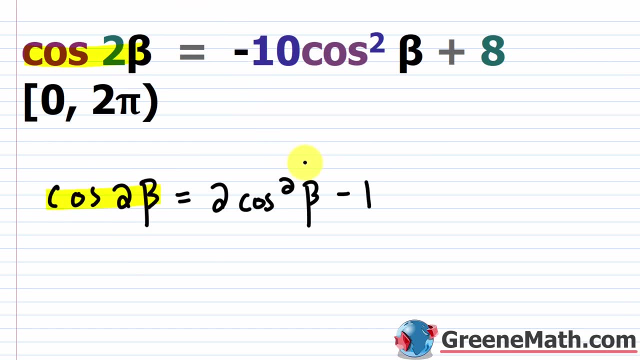 So I'm just matching this formula here. I'm just taking the beta in the place of beta And basically now you have cosine of 2 beta and cosine of 2 beta. So those match and what you can do is take this guy right here And you could just plug it in for this guy right. 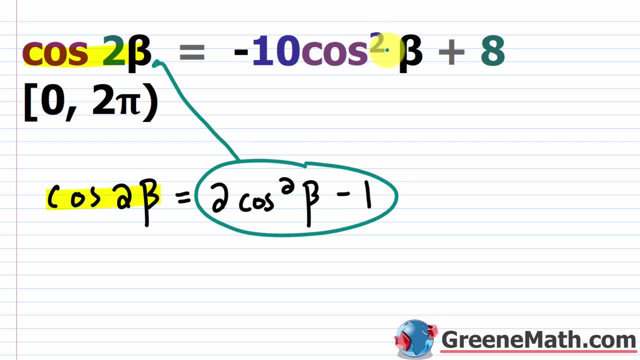 here, And that's going to give me cosine squared beta over here and cosine squared beta over here. So that's what I want. So let's write this as 2 cosine squared beta minus one again, just taking this and plugging it in for this. So that's how I get this left side now. So this equals on the right. 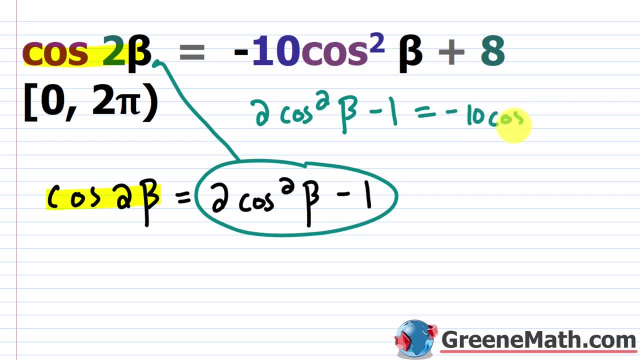 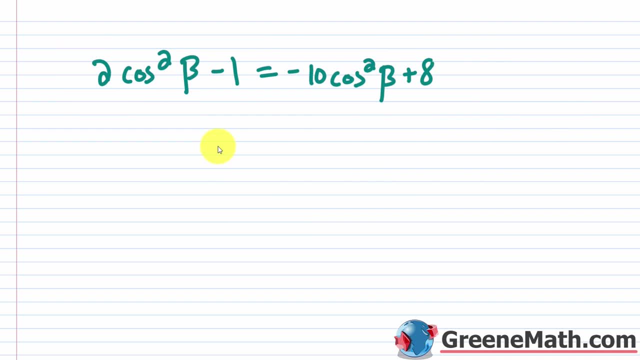 nothing's going to change. So this is just negative. 10 cosine squared beta and then plus eight. Okay, I want to get. cosine of beta equals some number. if you have a squared guy involved, then you should be thinking about factoring or, in some cases, the quadratic formula. But for 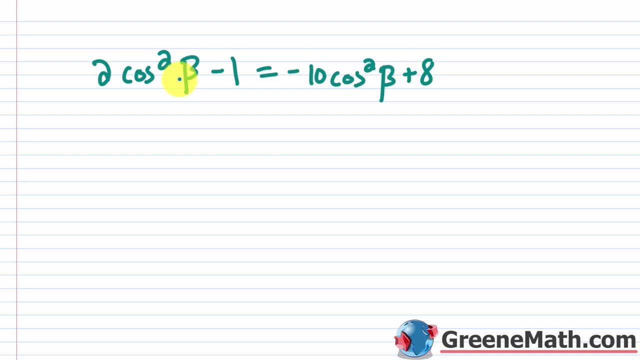 this particular problem. you could actually solve it using the square root property And it's going to be a lot faster. you could solve this with factoring if you want to, but it's going to take a little bit more time. So what I'm going to do is isolate cosine squared. 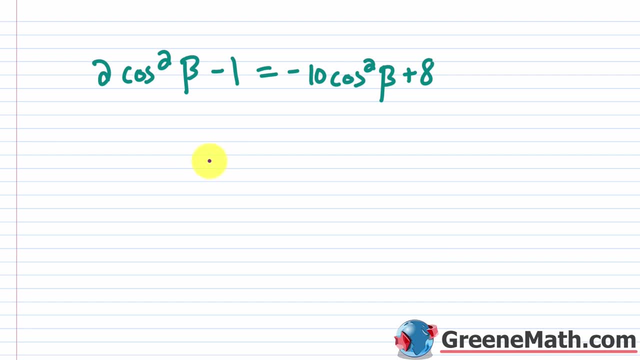 beta on one side and then have a number on the other side So I can use the square root property. So I'm going to add 10 cosine squared beta to both sides of the equation, just like that. And so, right here, this is going to cancel, And then the other thing I'm going to do is add one. 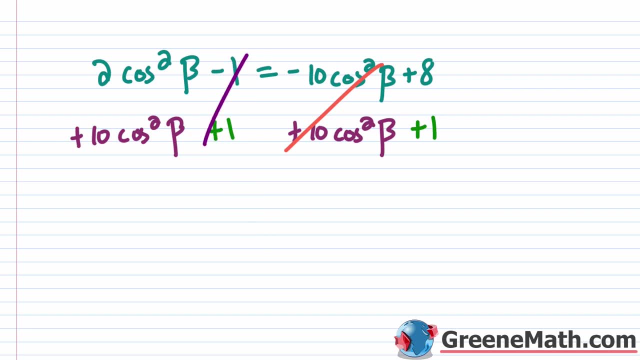 to both sides of the equation. So this is going to cancel. So on the left you have to cosine squared beta. then plus 10 cosine squared beta, that is 12 cosine squared beta, and this equals eight plus one. Now what you would want to do, since 12, is multiplying the cosine squared beta there. 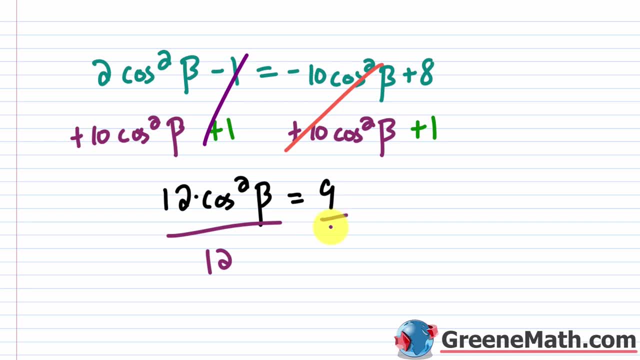 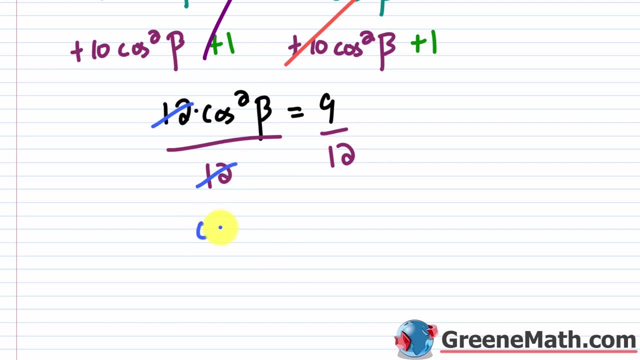 you would divide both sides of the equation by 12.. So you want cosine squared beta by itself to use the square root property. OK, so this right here is going to cancel and you get: cosine squared beta is equal to for 9 over 12.. 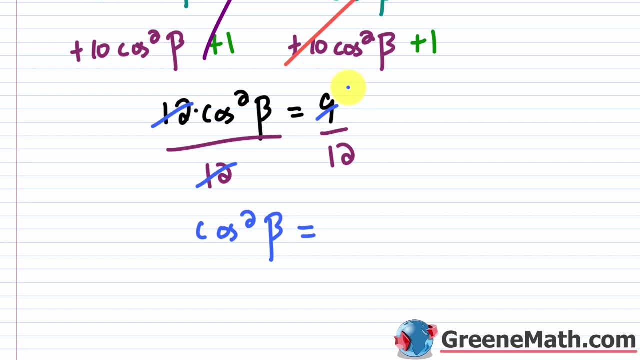 Again, each is divisible by 3.. So 9 divided by 3 is going to be 3, and 12 divided by 3 is going to be 4.. So this is: cosine squared beta is equal to 3 fourths, And now we can use our square root property. 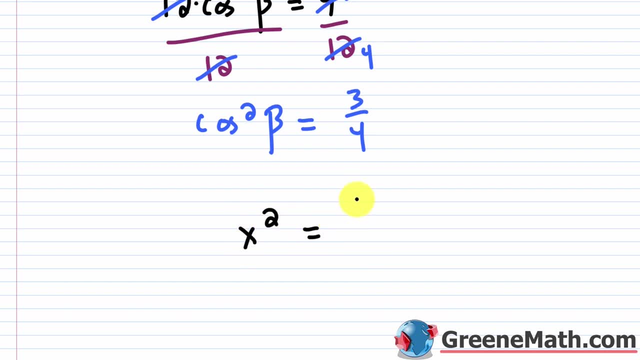 Again, if we have something like: let's say x squared equals 3 fourths, then by the square root property we can say: x is equal to plus or minus the square root of 3 fourths. So that's the square root of 3 over the square root of 4, which is 2.. 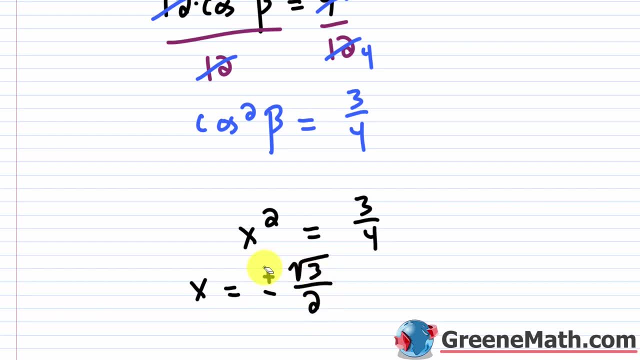 So x would be equal to plus or minus the square root of 3 over 2.. Well, here it's the same thing. I'm just going to get that. cosine Of beta is equal to plus or minus the square root of 3 fourths. 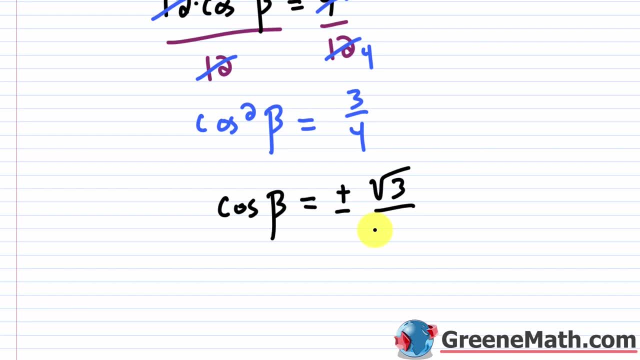 And again this becomes the square root here of 3 over the square root of 4.. And the square root of 3 really can't do anything with that, But the square root of 4 is going to be 2.. So the cosine of beta is equal to plus or minus the square root of 3 over 2.. 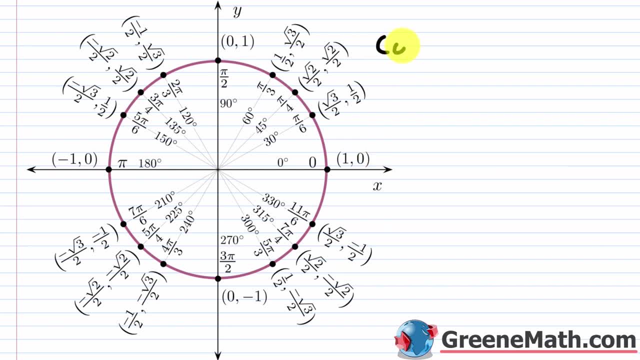 OK, let's come to the unit circle And let's actually write this: as the cosine of beta is equal to the square root of 3 over 2.. And then I'm going to write: or the cosine of beta Is equal to the negative of the square root of 3 over 2.. 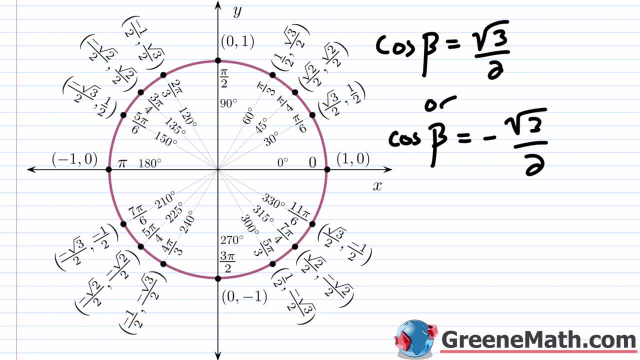 So for beta here we're going to look in quadrants 1 and 4, where cosine is positive, And I'm looking for an x coordinate of square root of 3 over 2.. So right here at pi over 6.. 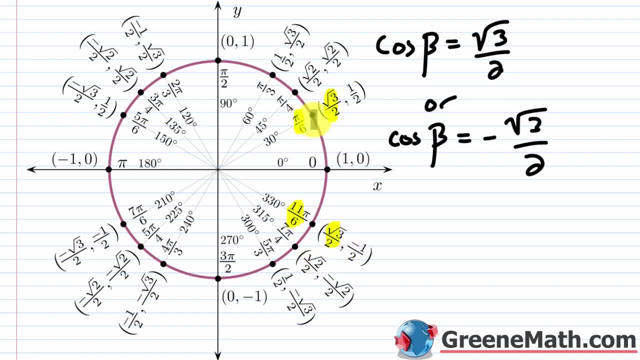 And then, coming down here, it's going to be at 11 pi over 6.. So notice it's pi over 6 here and then a pi over 6 reference angle here at 11 pi over 6.. Then if I'm looking for cosine of beta to be equal to negative square root of 3 over 2.. 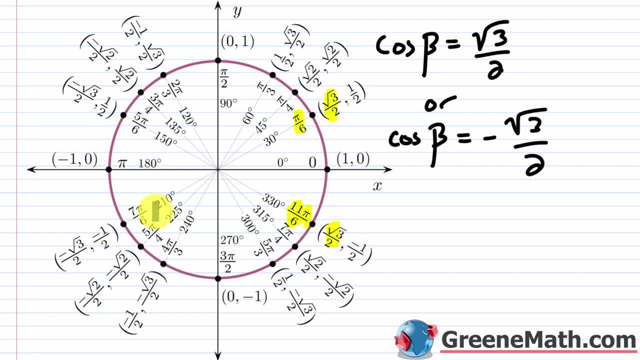 Well, I'm looking in quadrants 2 and 3, where cosine is negative. So you can just think about a Pi over 6 reference angle. or again, you could just look for that x coordinate of negative square root of 3 over 2.. 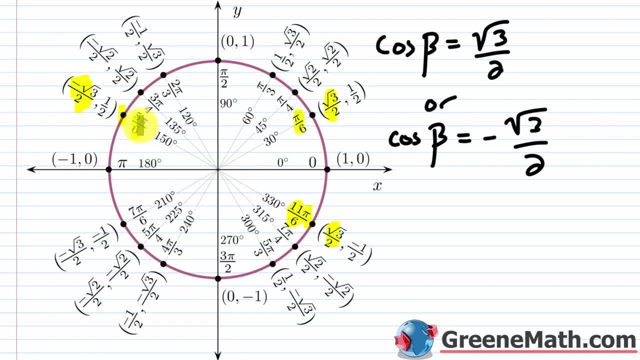 So that's going to be right here at 5 pi over 6, again pi over 6 reference angle, And then right here at 7 pi over 6, again pi over 6 reference angle. So because we're working in the interval where beta is greater than or equal to 0 and less than 2 pi, we can just list these four solutions and be done with it. 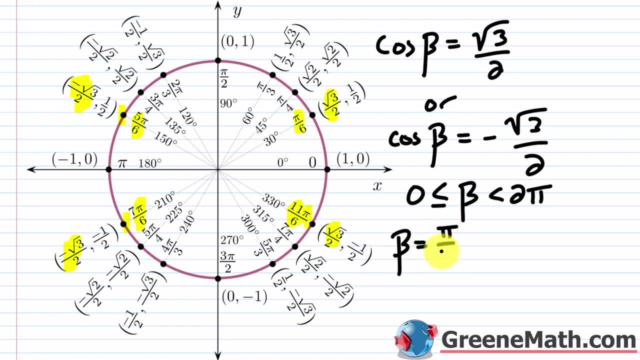 So we're going to say that beta is equal to: we have pi over 6.. We have 5 pi over 6.. We have 5 pi over 6.. And then we have 7 pi over 6.. And then, lastly, we have 11 pi over 6.. 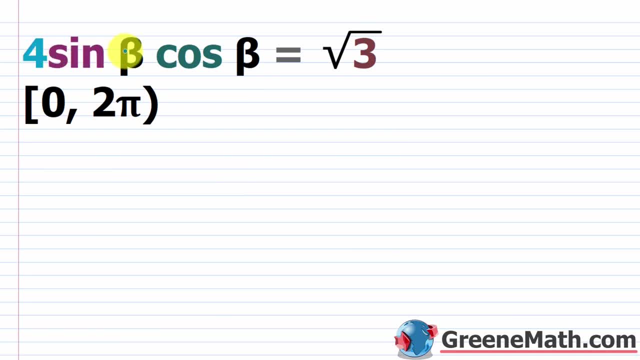 All right, let's take a look at the next problem. So here we have 4 sine of beta. cosine of beta equals the square root of 3.. We want to solve this over the interval from 0 to 2 pi, where 0 is included and 2 pi is excluded. 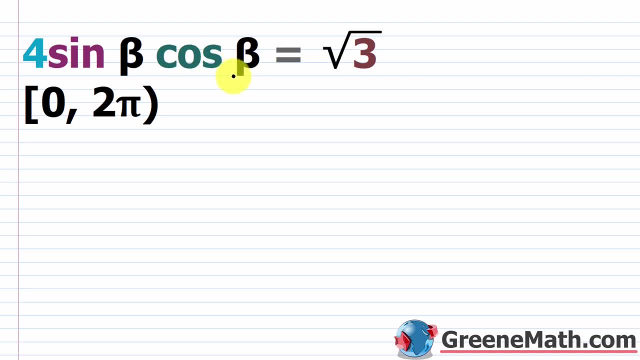 So the first thing is, when you look at this equation it might not be immediately obvious what you can do. But if we look at our identities again, you have something like this double angle identity- The sine of 2 theta equals 2 sine of theta, cosine of theta- which you can use to solve this equation. 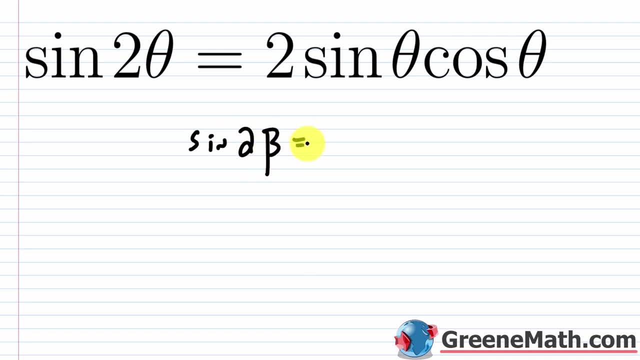 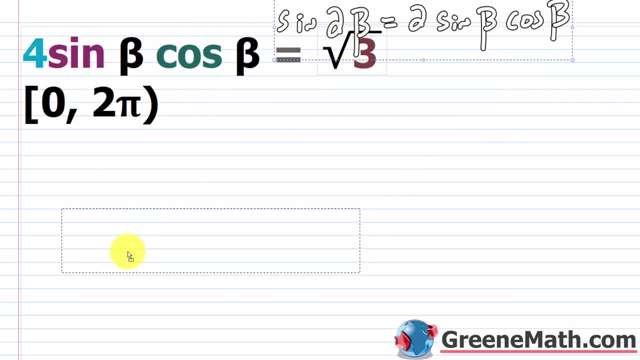 So I'm going to write this: as the sine of 2 beta is equal to 2 sine of beta, cosine of beta. Come back up here and paste this in Now. this might not be immediately obvious, but we're going to take this right here and match it with this right here. 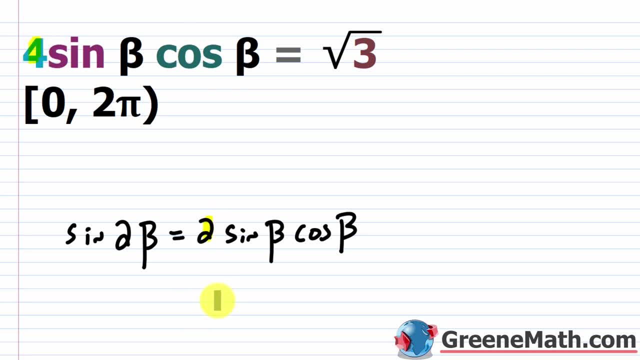 Now, right now you have this 4 right here and you have this 2 right here, So you've got to rewrite this to where it's going to match. So this is just straight Multiplication. So for 4, I could really write that as 2 times 2.. 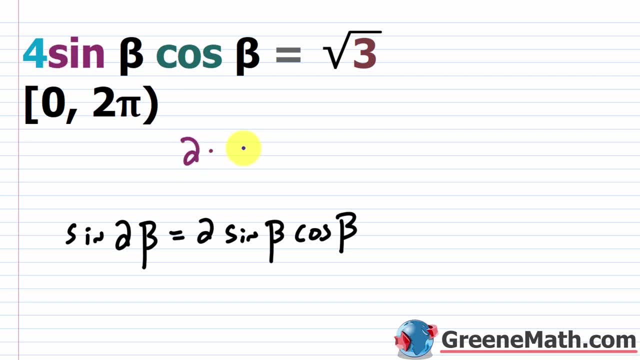 So I could say that this is 2 times, and then it would be 2 sine of beta- cosine of beta, And this equals the square root of 3.. So this 2 times 2 sine of beta- cosine of beta gets me back to 4 sine of beta- cosine of beta. 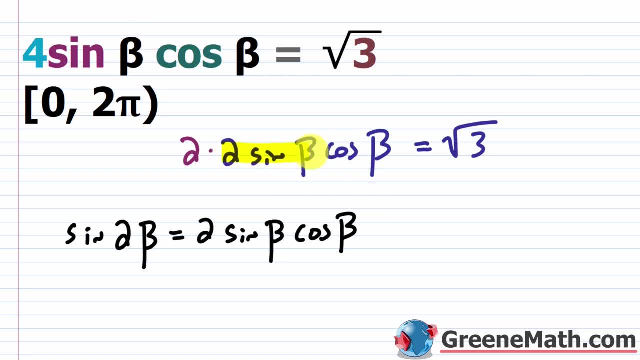 So I haven't done anything illegal. If you look at this guy right here now, it matches this guy right here perfectly: 2 sine of beta, cosine of beta. 2 sine of beta, cosine of beta. So that means I can legally take this right here and I can plug it in for this right here. 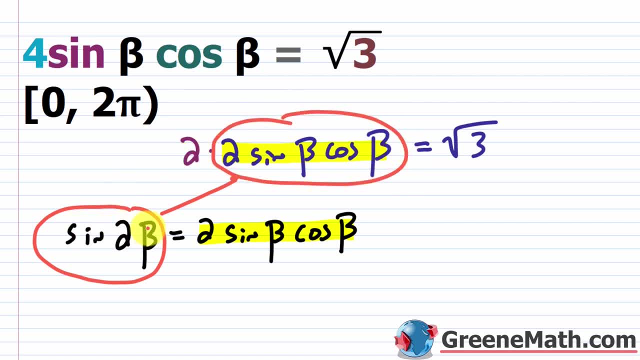 So what that's going to do for me is I'm going to have 2 sine of 2. beta equals the square root of 3.. So I'll be able to get it to sine of 2 beta equals some number and I'll be able to get a solution. 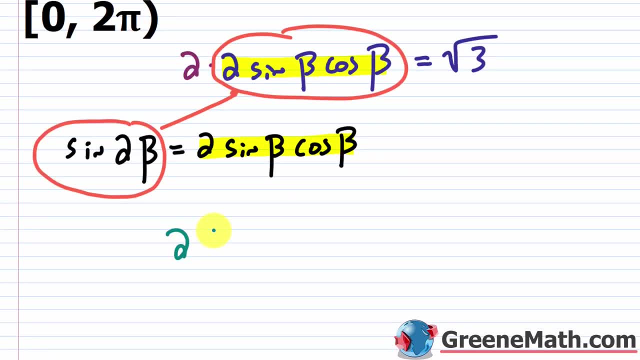 So let's go down and make a little substitution here. So I'm going to have my 2.. Don't forget about that. And then what is it multiplying Again for this? I'm plugging in this, So I'm going to have my sine of 2 beta. 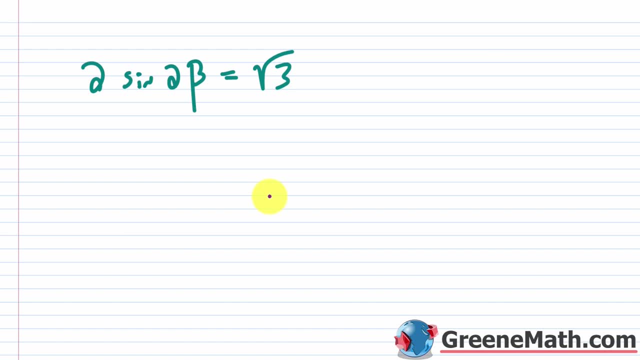 And this equals my square root of 3.. All right, So just like I said, we want to get sine of 2. beta equals some number. Right now you have 2. that's multiplying the sine of 2 beta. So let's divide both sides of the equation by 2.. 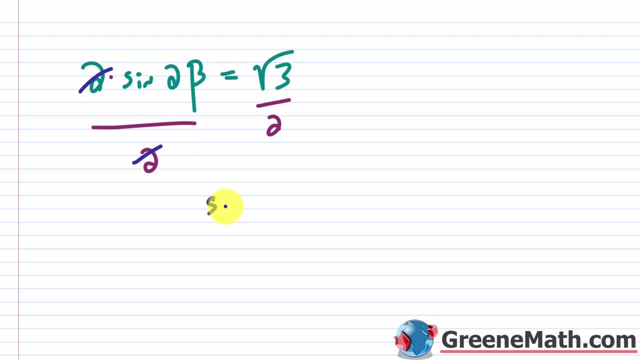 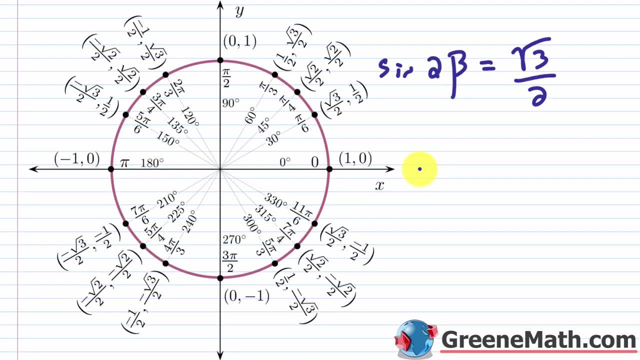 So this is going to cancel And we're going to get. the sine of 2. beta is equal to the square root of 3 over 2.. All right, There are quite a few ways you could solve this. What I'm going to do is stick to the method that the book uses, because we're solving over a specific interval. 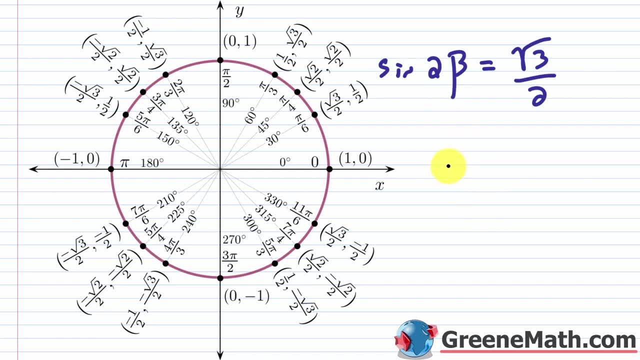 We're not giving the general solution, So I'm going to start with the integral we were given. So we have: beta is greater than or equal to 0 and less than 2 pi. Well, right now I have 2 beta, So I'm going to multiply each part of this inequality here by 2.. 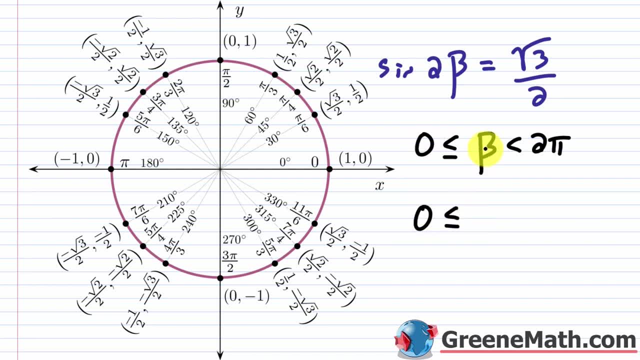 So 0 times 2 is still 0. And this is less than or equal to Beta. times 2 is 2 beta. So now this matches this, And then this is less than 2 pi times 2 is 4 pi. 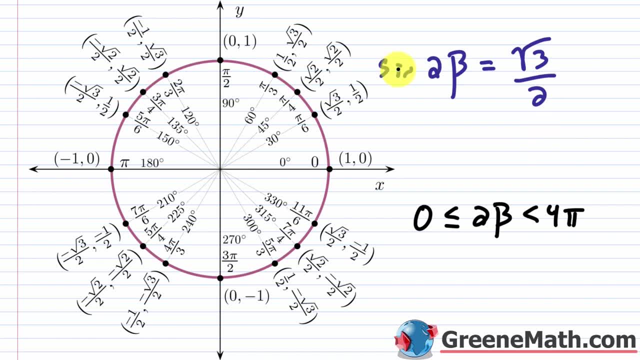 So right now, Okay, So I'm going to start with the integral we were given And I'm going to work in this interval because, again, I have the sine of 2 beta, not the sine of beta. So that's why I'm adjusting this interval. 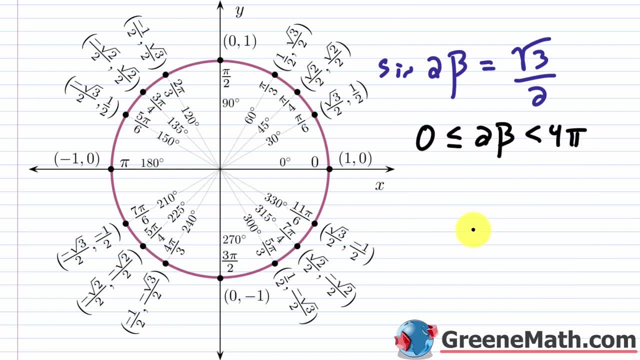 So let me move this up here And we're going to think about where are the sine values, square root of 3 over 2 in this interval, right here. So let's start with the standard interval. So just going from 0 to 2 pi. 0 included, 2 pi excluded. 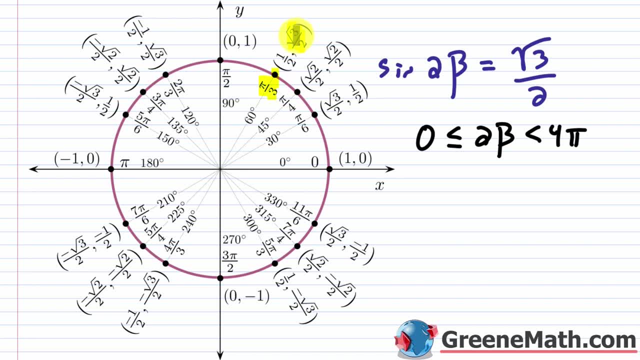 And that's going to give you a pi over 3 solution. So there's your square root of 3 over 2 for the y value, And then here's your square root of 3 over 2 for the y value as well. 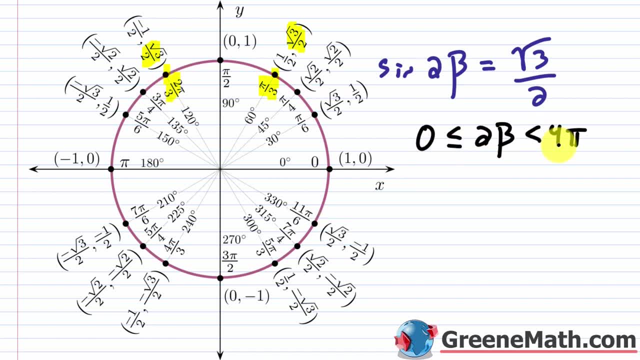 So that's at 2 pi. But again, to get all of the solutions in this interval, what you have to do is take those solutions and you have to add 2 pi to them in order to get all the solutions in this interval. 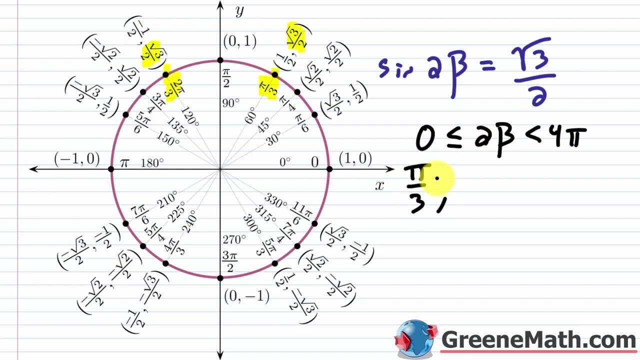 So I'm going to take and list pi over 3. And then let me list 2 pi over 3. And then what I would have to do is again take pi over 3.. So pi over 3. And I've got to swing around by another 2 pi. 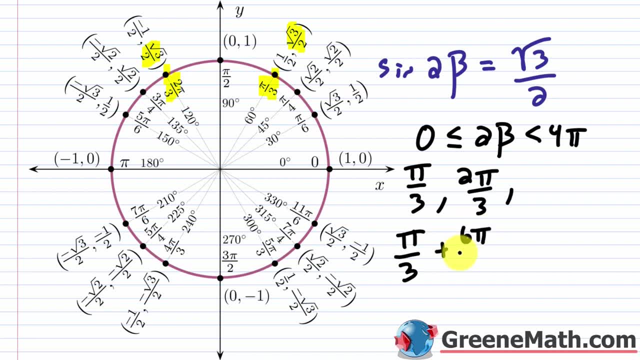 So let me go plus 2 pi, So that's 6 pi over 3.. If I get a common denominator, let me make that 3 a little bit better, So that's 7 pi over 3.. So let's put that up there. 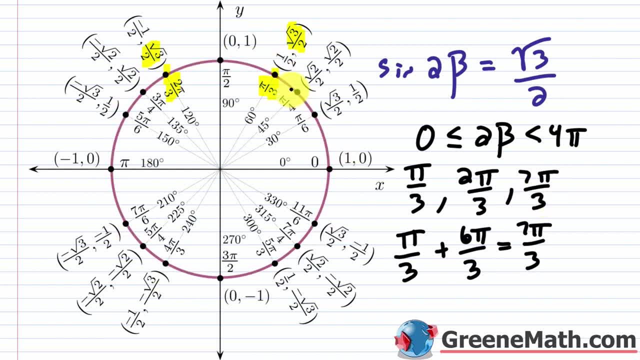 So that's 7 pi over 3.. So again starting here, just swinging around by another 2 pi. You've got to do the same thing here, So you're going to swing around by another 2 pi. So let's put this as 2 pi over 3, plus again 6 pi over 3.. 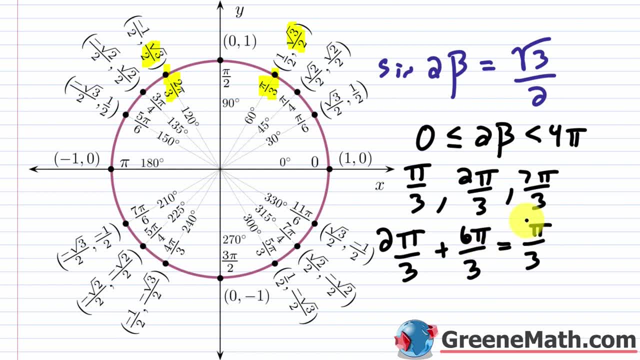 So 6 pi over 3 is again 2 pi, written with a common denominator. So this would be 8 pi over 3.. So 8 pi over 3.. So that's basically all you have to do For this part. 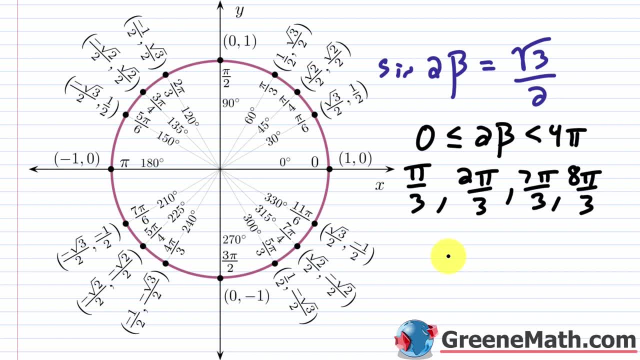 The only thing is you have not solved for beta, You've solved for 2 beta. So in other words, you could say that 2 beta is equal to this. right here, Let me just drag this down, And I don't know if that's going to fit. 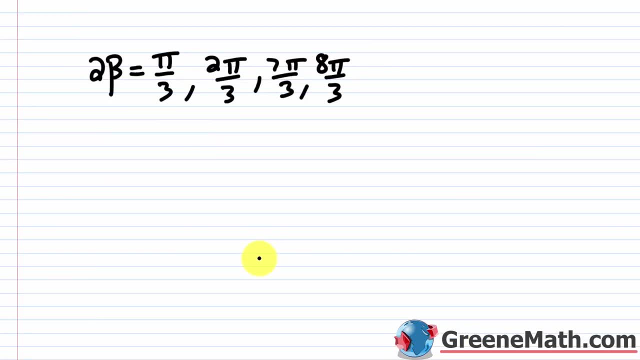 And let me just grab this real quick and paste this in and go to another page. So basically, if you want to solve for beta, you would divide everything by 2. Or you could multiply everything by a half. So in other words you could say that beta is equal to. 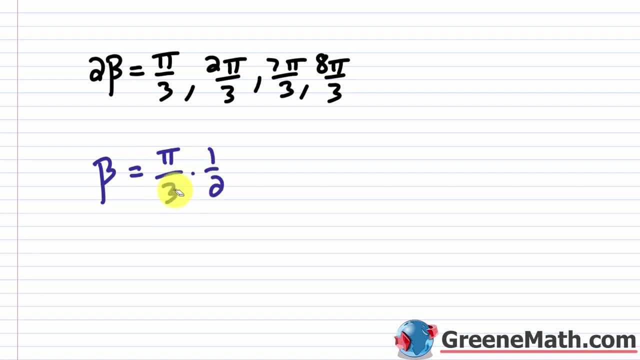 You'd have pi- Pi over 3 times 1 half, So that would be pi over 6.. So pi over 6.. And then you'd have 2 pi over 3 times 1 half, So the 2s would cancel there. 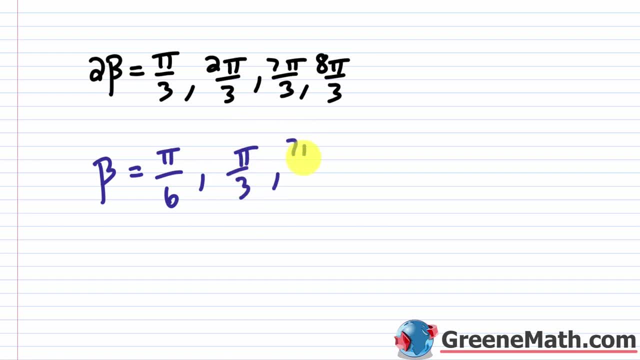 So that would be pi over 3.. So pi over 3. And then you'd have 7 pi over 3 times 1 half. That would give you 7 pi over 6.. And then, lastly, you'd have 8 pi over 3 times 1 half. 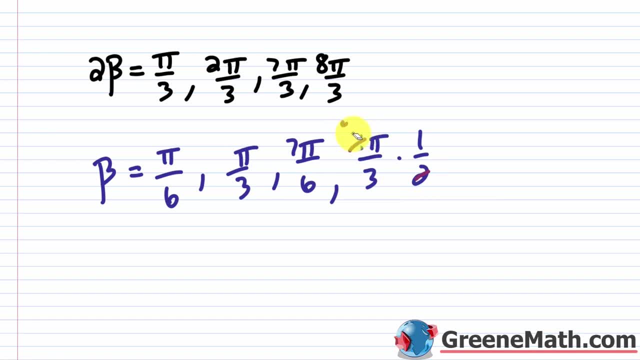 So here, 8 divided by 2 would give you 4.. So this would end up being 4 pi, So 4 pi over 3.. So these are your solutions in terms of beta. So if you plug those back into the original equation, they will work. 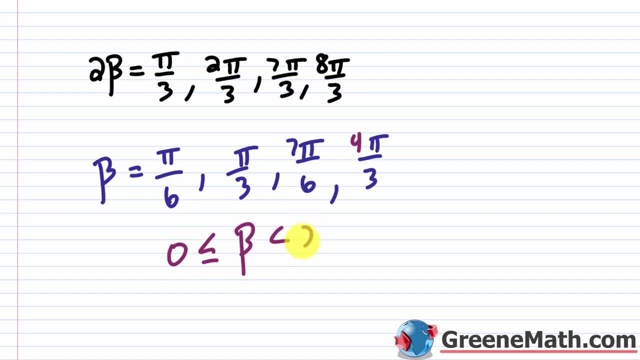 And they are in our interval where beta is greater than or equal to 0 and less than 2 pi. So beta is pi over 6,, pi over 3,, 7 pi over 6, and then 4 pi over 3.. 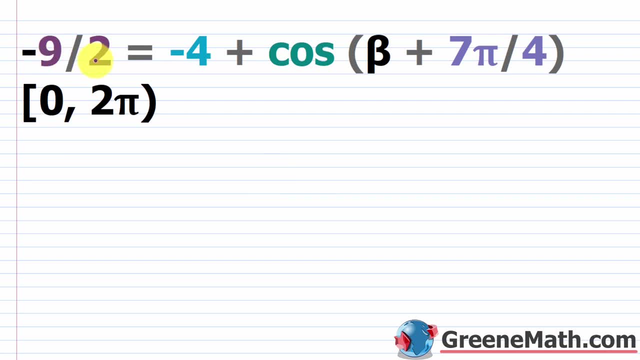 All right, let's take a look at another problem. So we have negative 9. halves is equal to negative 4 plus the cosine of beta, plus 7 pi over 4.. We're solving this over the interval from 0 to 2 pi. 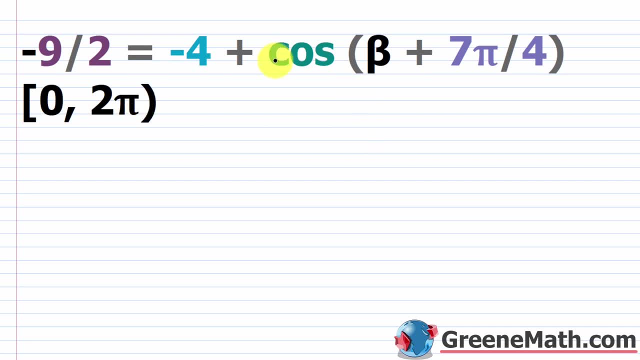 Where 0 is included and 2 pi is excluded. So I'm going to get cosine of beta plus 7 pi over 4 by itself. So that'll be on one side. There'll be a single number on the other side. So that's the first goal. 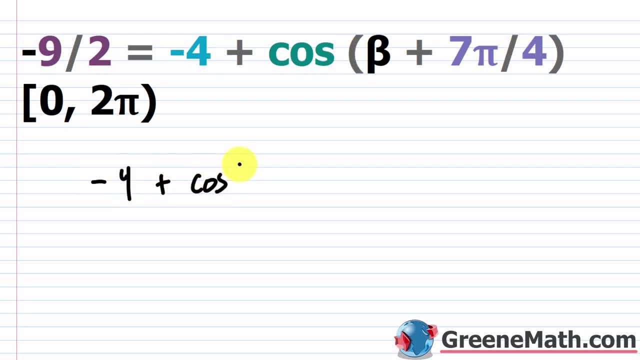 So let me write this as negative 4 plus cosine of beta plus 7 pi over 4.. And then this would be equal to. you have this negative 9 halves. Now, if I want cosine of beta plus 7 pi over 4 on one side by itself. 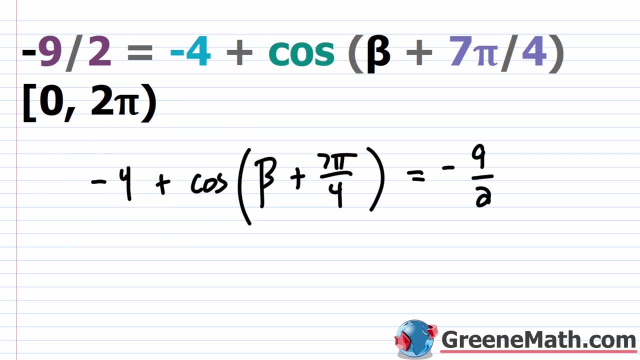 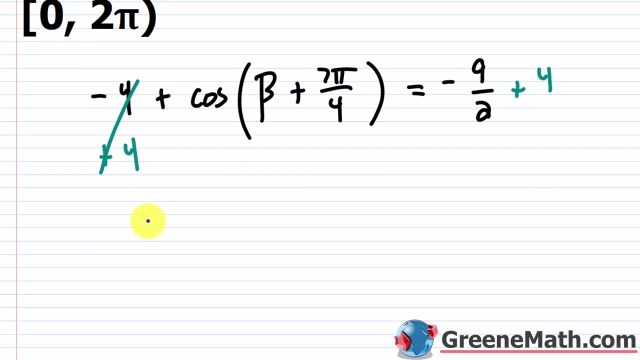 I've got to get rid of this negative 4 here That I'm adding to this. So I'm going to just add 4 to both sides of the equation. This will cancel And on the left I have what I want. 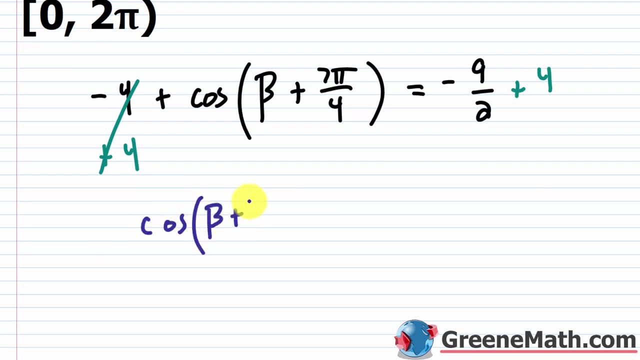 So this is the cosine of this beta plus 7 pi over 4.. And this equals over. here I would get a common denominator. So let's write 4 as 8 over 2.. I'm just going to multiply by 2 over 2 to do that. 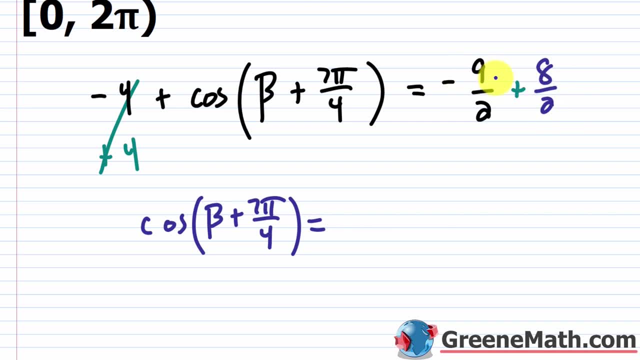 So again this would be 8 over 2.. So 8 over 2 and negative 9 plus 8, that's negative 1. So this would be over the common denominator of 2. So this is equal to negative 1 half. 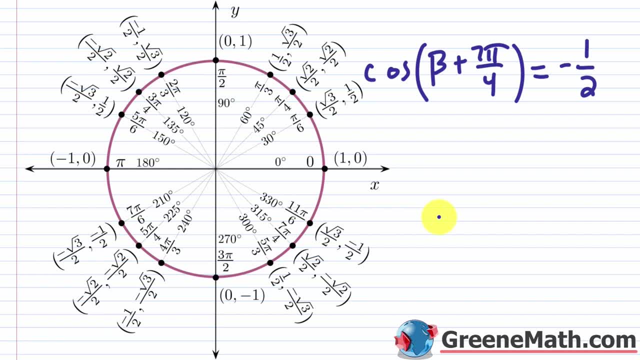 Now this is the part where people tend to get confused. Essentially, what you're going to do is adjust your interval. You don't have beta. So if you are solving, cosine of beta equals negative 1 half, well then I could go through and I could say: well, where's the x-coordinate? 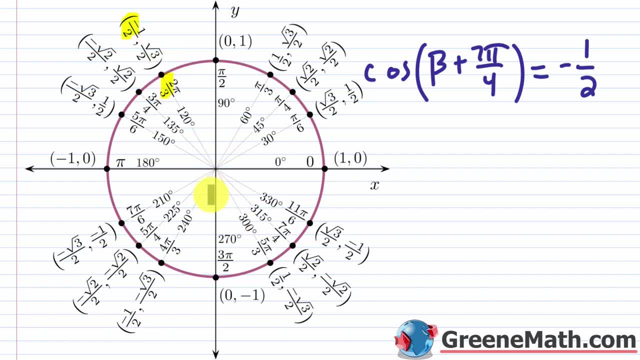 negative 1 half we're going to have right here at 2 pi over 3.. And then you come over here and that's going to be at 4 pi over 3.. We don't have that, though. We have this beta plus 7 pi over 4.. 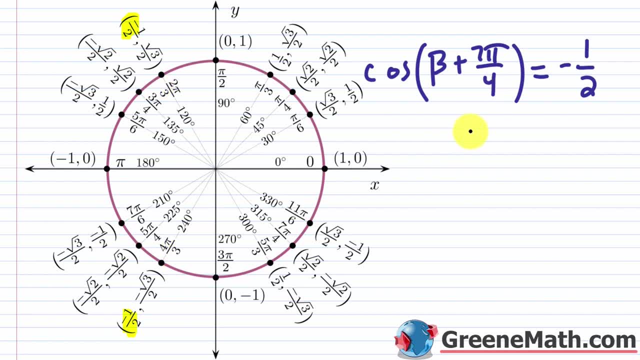 We don't have beta. Well, I can adjust that interval We had. beta is greater than 4 pi over 3.. Greater than or equal to 0 and less than 2 pi. Well, instead of beta, I have beta plus 7 pi over 4.. 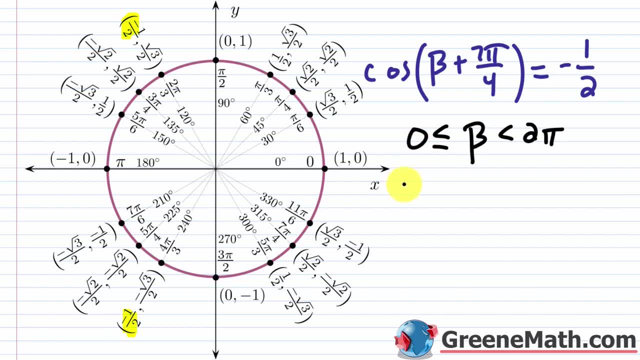 OK, well, I'm just going to add 7 pi over 4 to each part. So 0 plus 7 pi over 4 is 7 pi over 4.. This is less than or equal to, beta plus 7 pi over 4 is beta plus 7 pi over 4.. 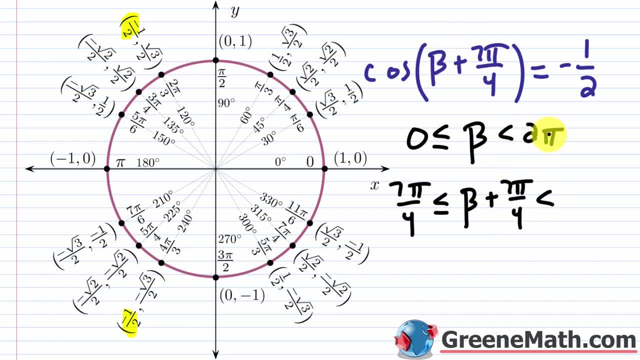 So this matches this, and this is less than 2 pi plus 7 pi over 4.. So if we do 7 pi over 4 plus let's go 8 pi over 4.. Just writing 2 pi with a common denominator, this would be 15 pi. 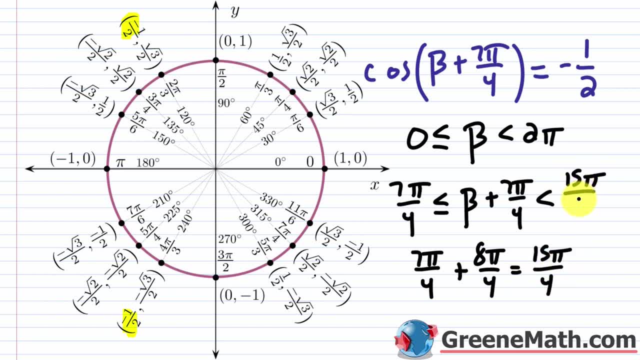 So 15 pi over 4.. So 15 pi over 4.. So if we had cosine of beta equals negative one half again, I would have this 2 pi over 3 and this 4 pi over 3. But in this case we have the cosine of beta plus 7 pi over 4.. 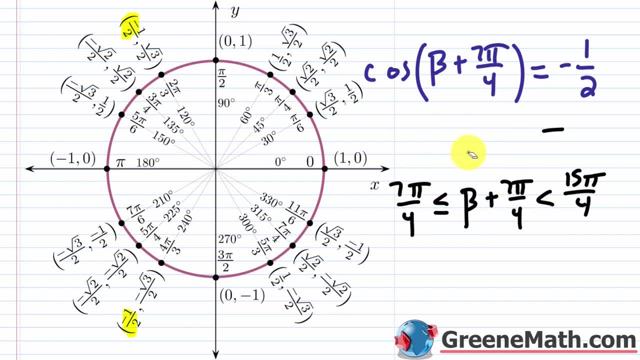 So when I adjust this interval to this one right here, let me get rid of this one right here. So this is crystal clear. What I'm going to do is look for where the cosine value is negative one half in this interval. So you would start. 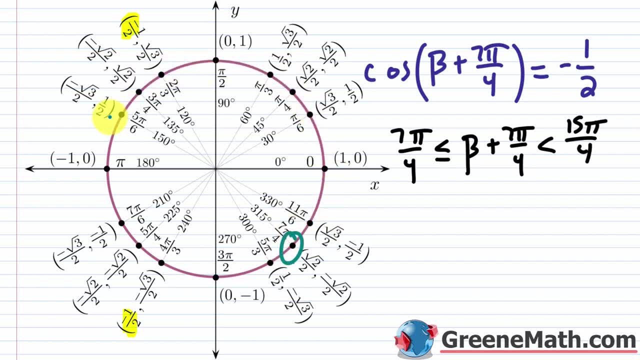 At 7 pi over 4.. So, in other words, you've already swung around by 7 pi over 4.. And then you want to swing around by another 2 pi to end up at 15 pi over 4, even though that's not included. 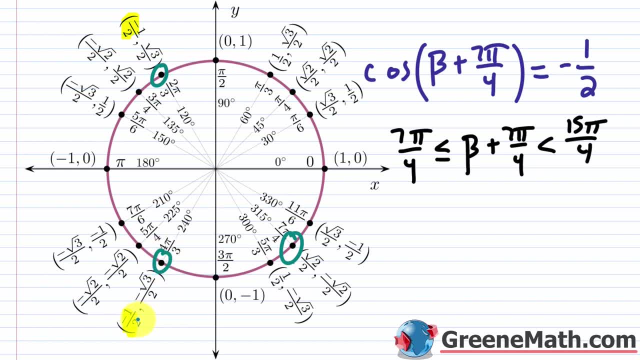 So you're going to catch this guy right here and this guy right here again, But it's not going to be 2 pi over 3 or 4 pi over 3.. It's going to be you adding 2 pi to those angles. 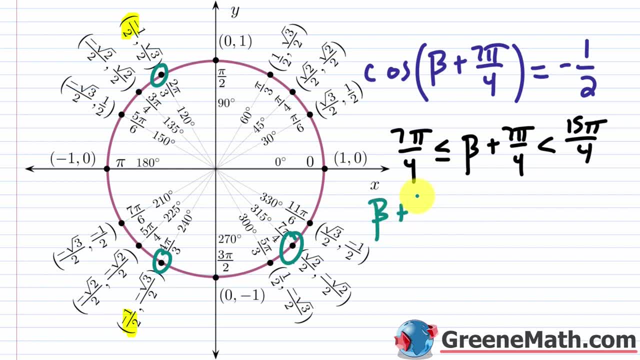 So what you would do is you would say that beta plus 7 pi over 4 would be equal to. you're going to take this 2 pi over 3. So 2 pi over 3. But now you've got to add 2 pi to that. 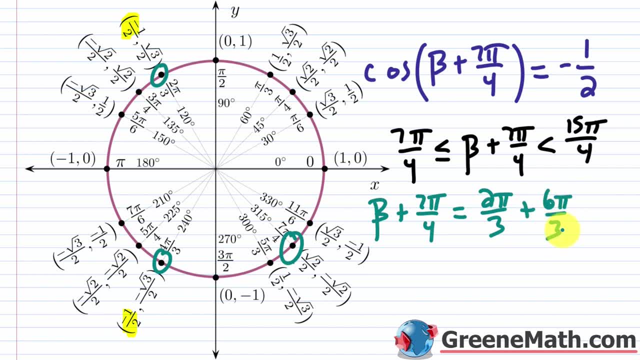 So that's going to be me adding 6 pi over 3. So that would give me 8 pi over 3. So you can get rid of these middle steps here and just say this is equal to 8 pi over 3.. 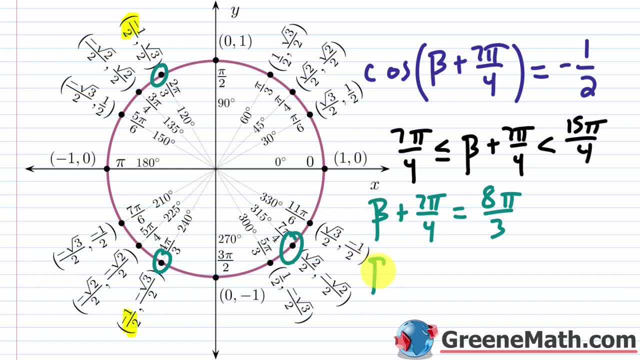 We'll solve this for beta in a moment. Let's just do the other one. So then again you have this beta plus 7 pi over 4 is equal to again, you're going to take this 4 pi over 3.. 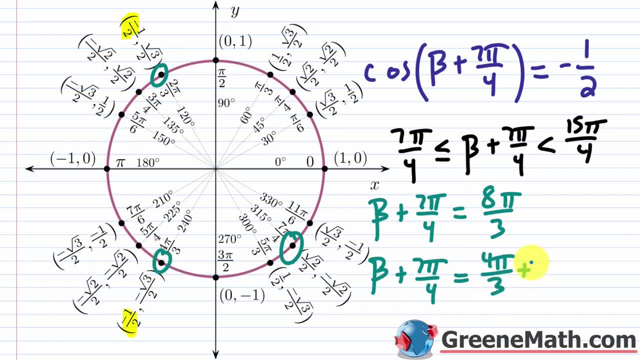 So this 4 pi over 3, and then you're going to add 2 pi, So you're going to say this is plus 6 pi over 3.. So this gives you 10 pi over 3.. Let me move this down here. 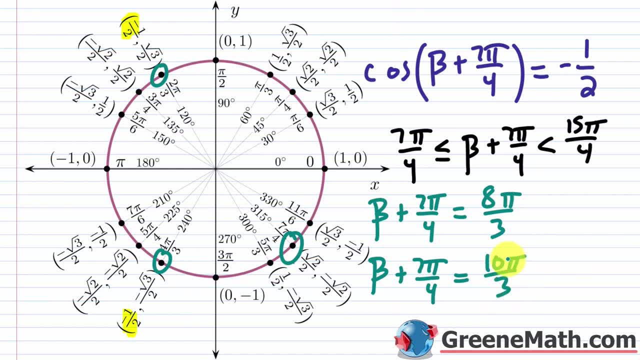 So this is more clear Now. I know the first time you do this. this is super confusing, But just think about the fact that again, you started here at 7 pi over 4.. That's where the interval is beginning. So if I'm starting here, by the time I swing around this is not 2 pi over 3.. 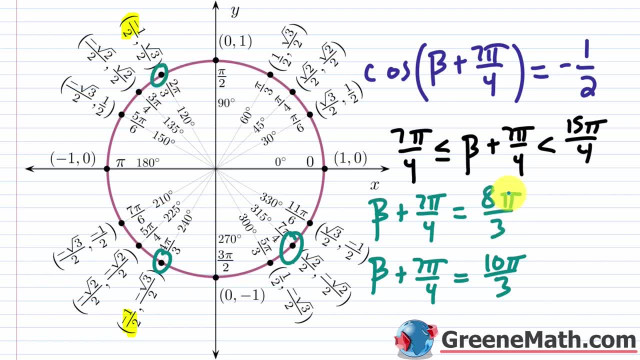 This is 2 pi over 3. Plus 2 pi, So that gives me that 8 pi over 3.. And then, as I continue, this is not 4 pi over 3.. This is going to be 4 pi over 3, plus 2 pi. 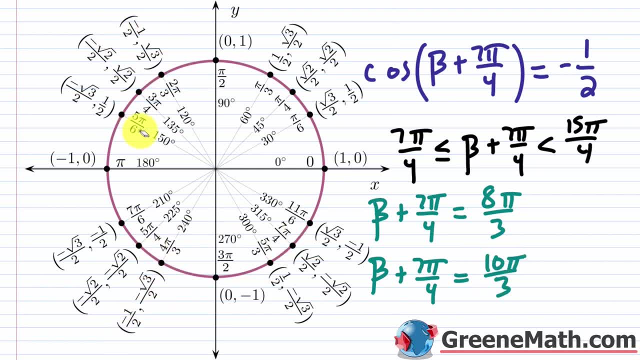 So that's that 10 pi over 3.. So you've got to adjust things, because we're not solving cosine of beta equals negative one half. We are solving cosine of beta plus 7 pi over 4 equals negative one half. So everything got adjusted. 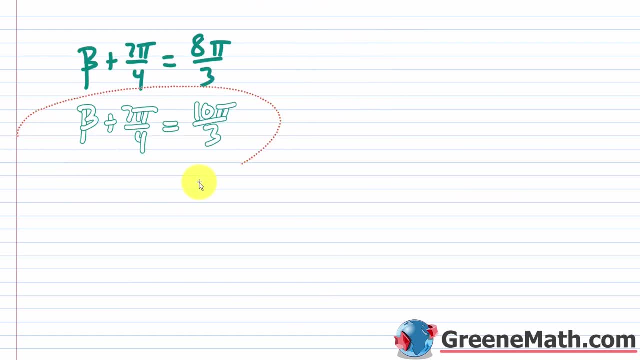 So let's go ahead and grab this And I'm just going to come down here and we can solve these pretty easily. Let's go over there. I'm going to subtract 7 pi over 4 away from each side of the equation over here. 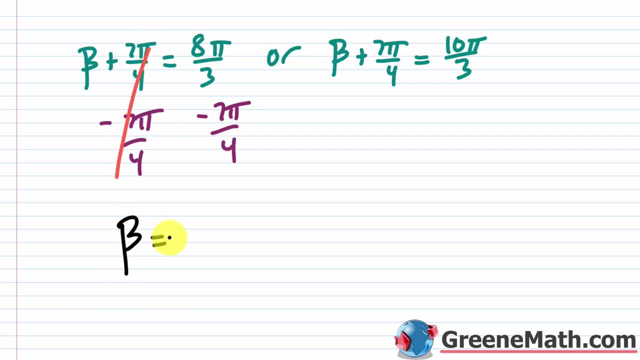 So this is going to cancel. You're going to have. beta is equal to 8 pi over 3 and then minus 7 pi over 4.. You need a common denominator, So let's multiply by 4 over 4.. Let's multiply this by 3 over 3.. 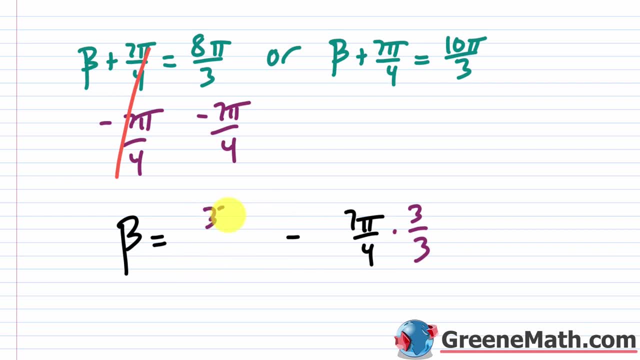 So this would be 32 pi over 12.. So 32 pi over 12, 21 pi, So 21 pi over 12.. So this would give me 7 pi, So 11 pi over 12.. So that's one solution. 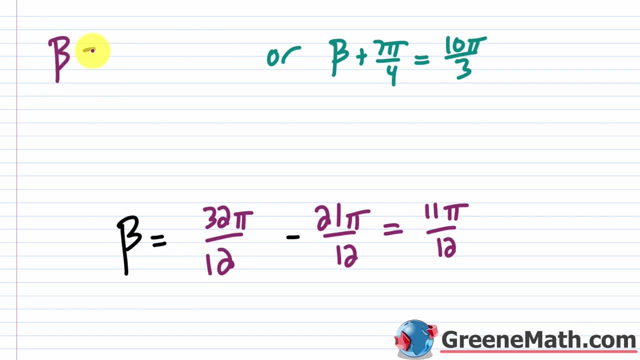 Let me get rid of this and just write this, as beta is equal to 11 pi over 12.. And let me solve this one now. So I'm going to subtract 7 pi over 4 away from each side of the equation, So that cancels. 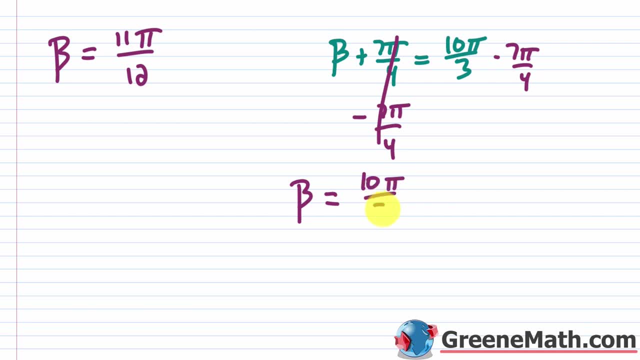 You get, beta is equal to- let's go- 10 pi over 3.. I'm going to just multiply this by 4 over 4 now to get a common denominator, and then minus 7 pi over 4 times 3 over 3.. 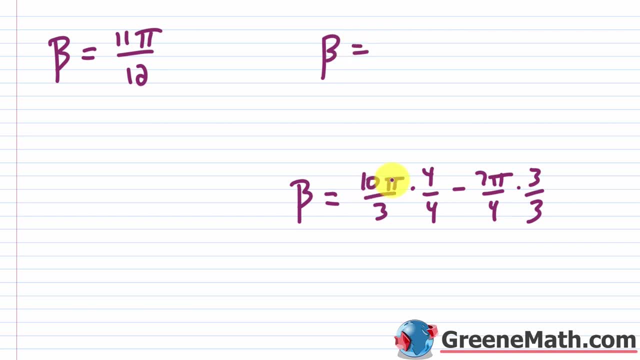 So we will say that beta is equal to 10 pi times 4 is going to be 40 pi, And this is over 12, and then minus 7 pi times 3 is 21 pi. So 21 pi And this is over 4 times 3 is 12.. 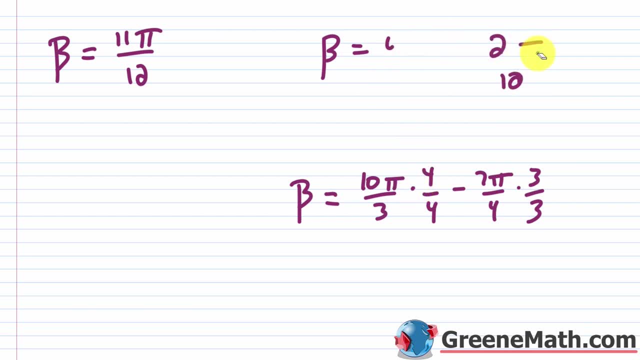 So 40 pi minus 21 pi is 19 pi. So this is 19 pi over 12.. Let me just put a comma here and put 19 pi over 12.. So those are your solutions in that given interval. Again, where beta is greater than or equal to 0 and less than 2 pi. 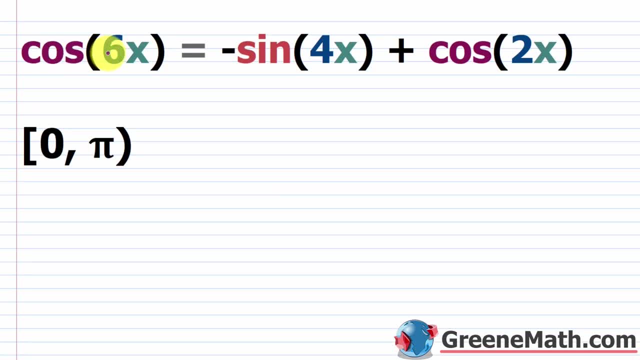 Okay, Let's take a look at another problem. So here we have: the cosine of 6x is equal to negative sine of 4x, plus the cosine of 2x. So here we're going to solve over this interval from 0 to pi, where 0 is included and pi is excluded. 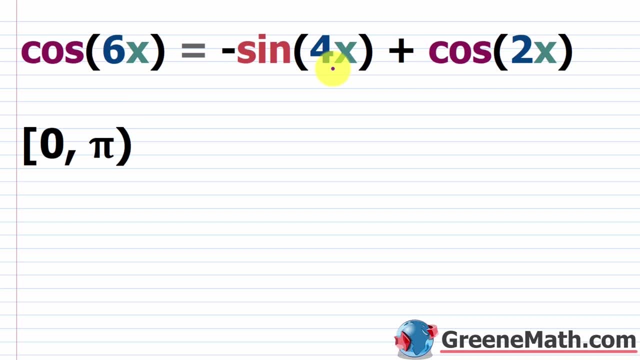 When you solve a problem like this that involves these sum to product identities. in most cases you're not going to solve that over an interval because there's just too many solutions. You will give the general solution. Let me start this problem off as saying: we have the cosine of 6x. 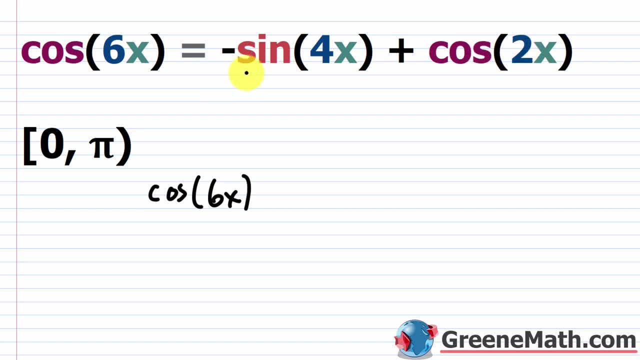 I'm going to add the sine of 4x to both sides and I'm going to subtract the cosine of 2x away from each side. So let me subtract away the cosine of 2x first, So I have this, and then I'm going to add sine of 4x and then we're going to say this equals 0. 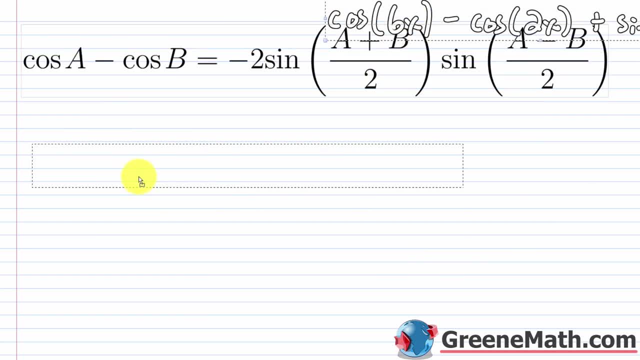 Okay, let's grab this real quick and let's come down here. So I have our little identity set up for us. So these are the again sum to product identities. So we have this cosine of A minus cosine of B, Cosine of 6x. 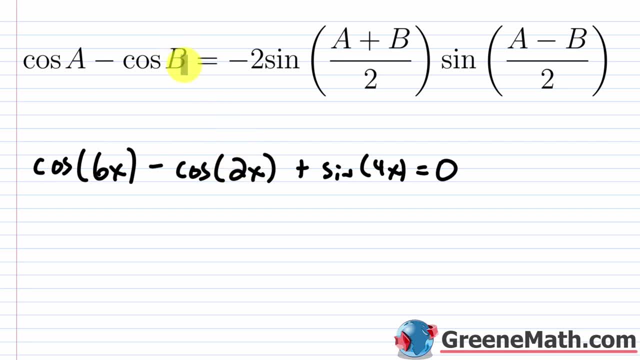 So 6x is your A, minus cosine of 2x, So 2x is your B. Let me actually slide this down and I'll write this out first and then we'll plug in. So if you add the cosine of 6x minus the cosine of 2x, 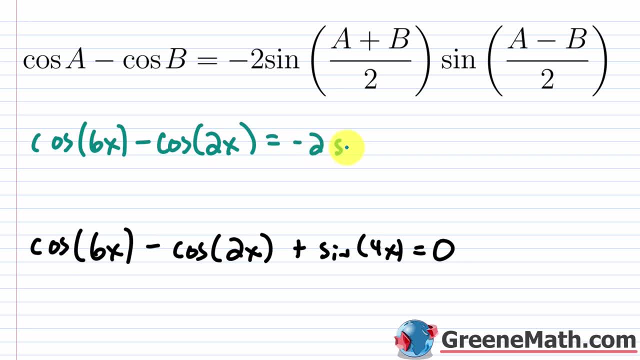 So I'm just going to do this part right here. This is equal to negative 2, and then sine of, you have A plus B over 2.. So this plus this, So 6x, 6x plus 2x over 2.. 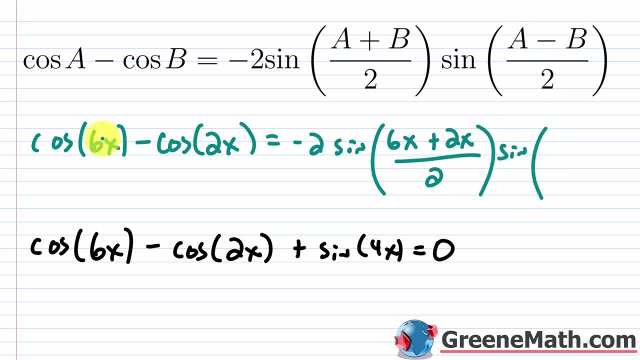 And then you have your sine of A minus B over 2. So 6x minus 2x. So 6x minus 2x Again, this is over 2.. 6x plus 2x is 8x. 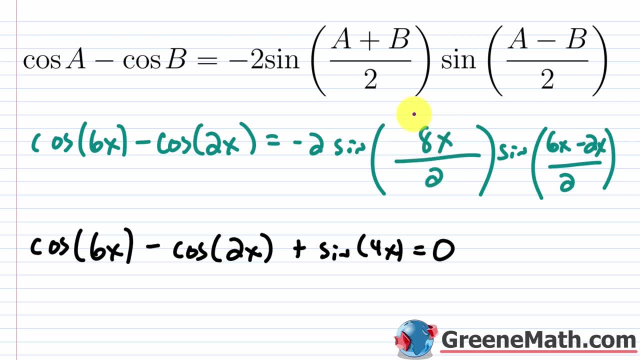 So this right here would be 8x over 2.. So this 8 would cancel with this 2 and give me a 4.. So this would be 4x right here. So let's write that like that. I'm just going to wrap this for clarity. 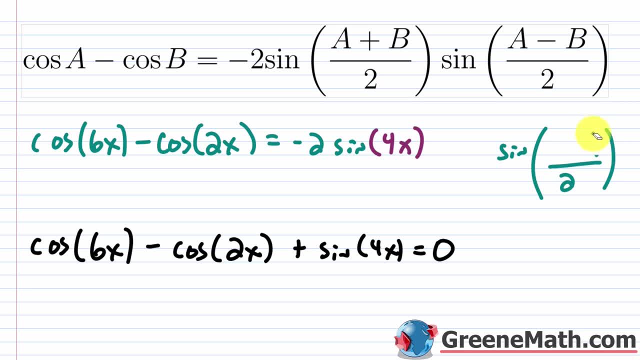 And then here, 6x minus 2x is 4x, And so this would be 4x over 2,, which is 2x. So let's write the sine of 2x Now, since this right here matches this right here. 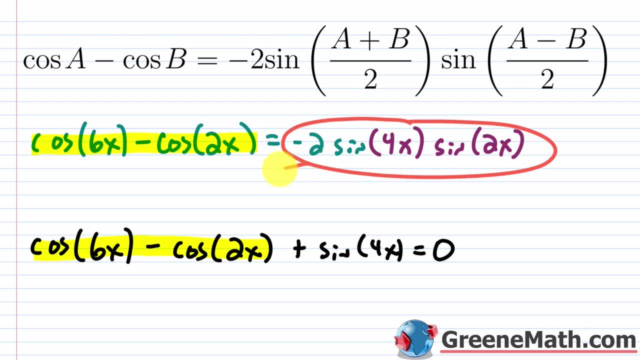 we can take this guy right here and plug it in for this right here. Now why are we doing that? Notice you'd have a sine and a sine, and then you have a sine And, more specifically, you have this 4x here and this 4x here. 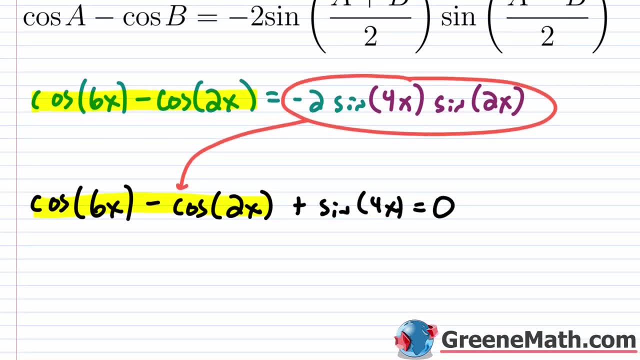 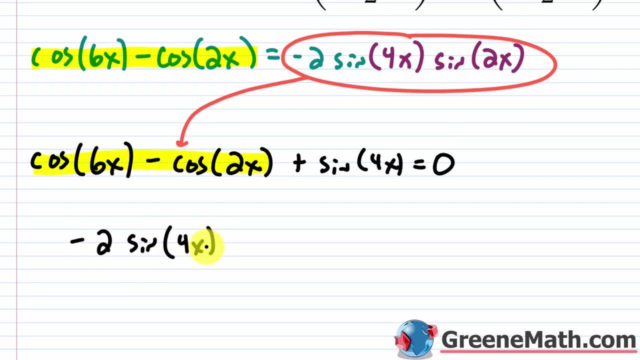 So we're going to be able to actually solve this with factoring. So let's come down a little bit and let's plug in. So this goes in here: So negative 2 and then sine of you have your 4x, and then sine of you have your 2x. 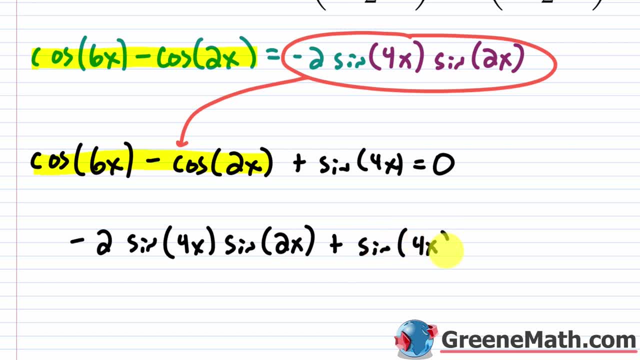 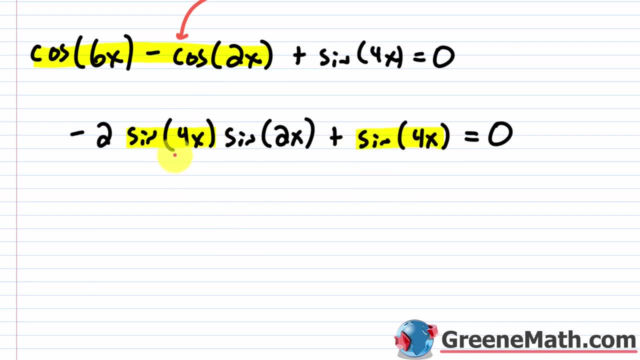 and then plus your sine of 4x, and this equals 0. So you have your sine of 4x and your sine of 4x. So we are going to factor that out. So let's factor that out. So, out in front of some parentheses, you would have the sine of 4x and then inside. 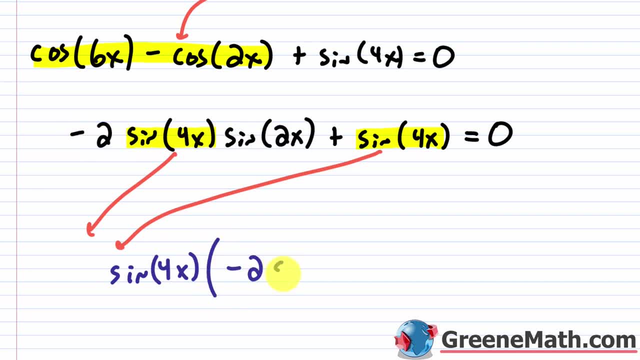 you would have negative 2 sine of 2x, So negative 2 sine of 2x, and then, plus, if this gets pulled out, you're going to have a 1, and then this equals 0.. Now, at this point, you can use your zero products property. 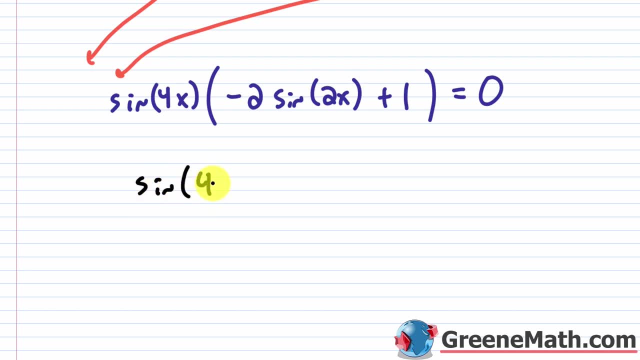 So you can say that the sine of 4x is equal to 0, or we're going to do this one. So negative 2 sine of 2x plus 1 equals 0. In this particular case, you have sine of something. 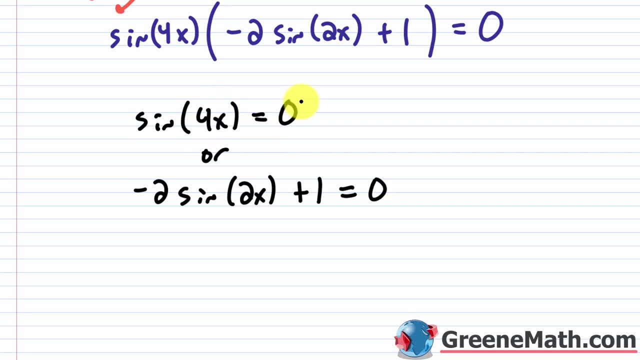 It doesn't matter what it is. In this case it's 4x. It's 2x equals 0 or some number. This is OK for this. When you want to clean it up, you would want sine of 2x equals some number. 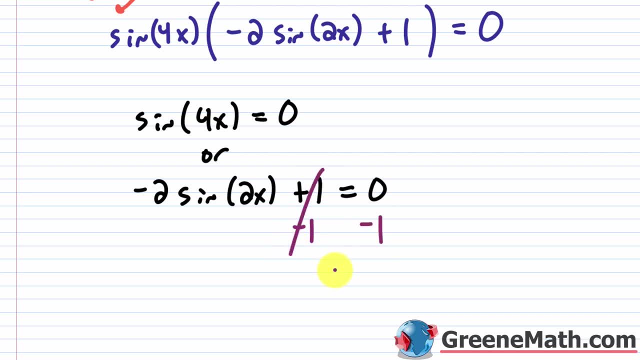 So let's go ahead and subtract 1 away from each side. This cancels, So actually let me just erase it so we can save some space here, And then I would divide both sides by negative 2. So this would cancel. 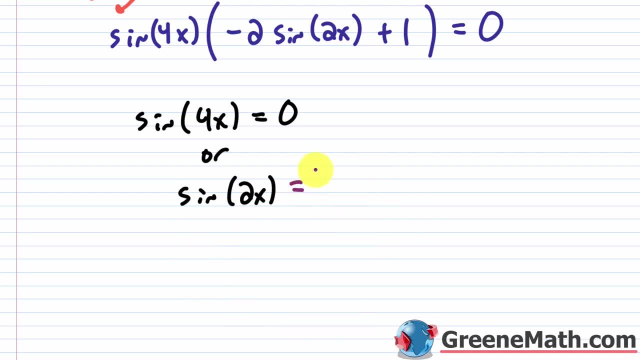 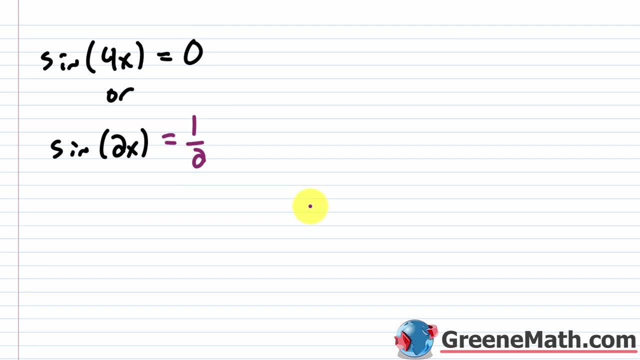 So you're going to get. the sine of 2x is equal to one half, So positive one half. Now here's where you need to make a decision Again. in most cases, you're going to solve for the general solution. 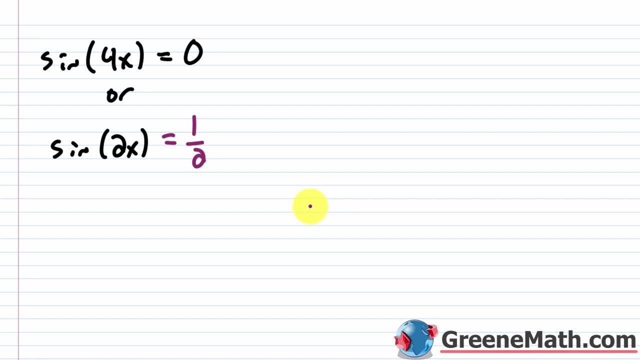 And when I solve for the general solution, I like to use a substitution technique, So you can do it this way if you want. If you're solving over an interval, you can do it the normal way that we've been doing it, by adjusting our interval. 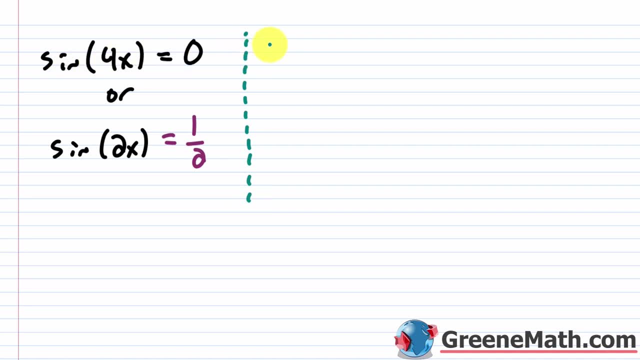 So, instead of sine of 4x equals 0, for this particular one, I'm going to let u be equal to 4x. Now, this has nothing to do with this, So actually, let me cut this away and put this on another page so nobody's lost, because people will get confused. 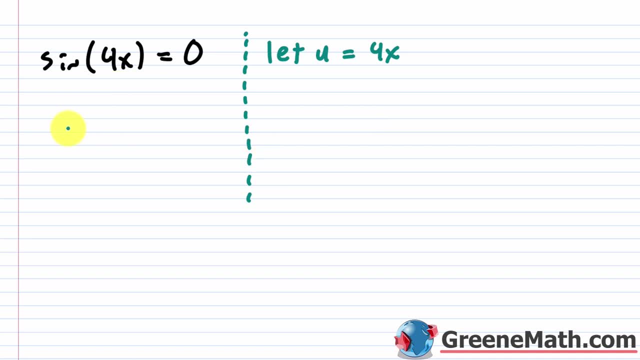 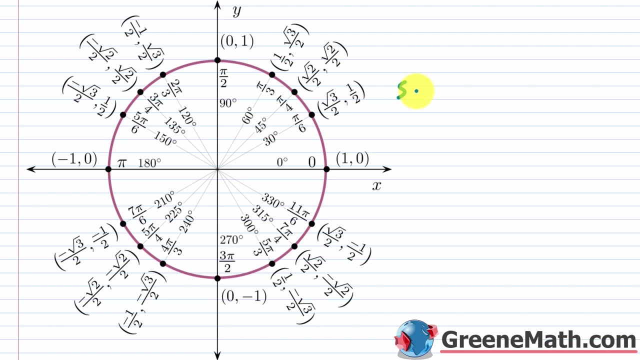 So now I can solve this. Let me get rid of this. Or by saying that I have: the sine of u is equal to zero. So if I look at, the sine of u equals zero using my unit circle, let me write this in: 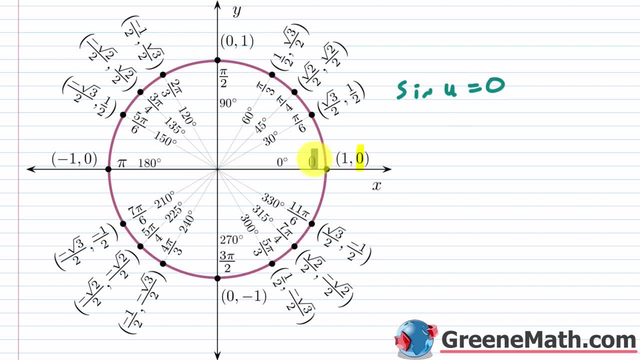 So the sine of u equals zero. So if you look at, this guy is zero, So that's at zero. And then this guy is zero, That's at pi. So you could write that u, in terms of the general solution, is equal to zero plus 2. 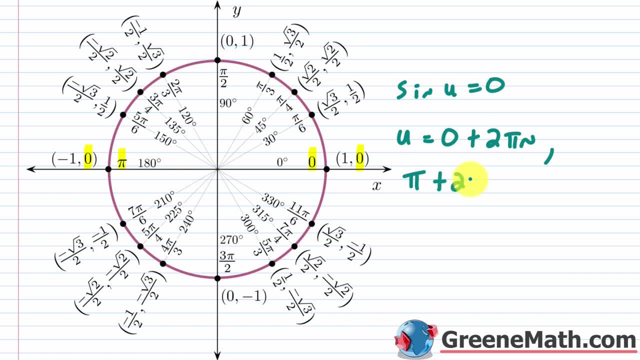 pi n, and then you could say pi plus 2 pi n, where n is any integer, because things are going to repeat every 2 pi in terms of u. Now what you could actually do is write this as 2 pi n, and then pi plus 2 pi n. 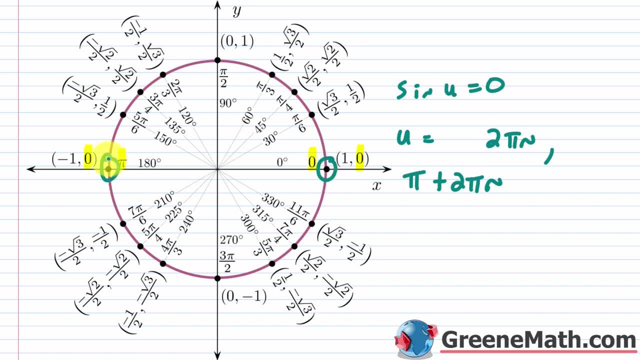 But you would notice that actually you can combine those solutions and make it a little bit more concise, because things are happening every pi. So in other words, I could just write this as pi? n. So I could write this as pi? n, because if I plugged in a zero for n, I'd have zero. 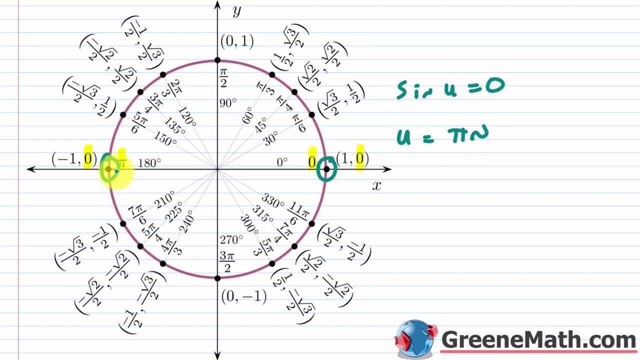 If I plugged in a 1,, I'd have pi. If I plugged in a 2,, I'd have 2 pi. At 3,, I'd have 3 pi, so on and so forth. So this is the general solution in terms of u. 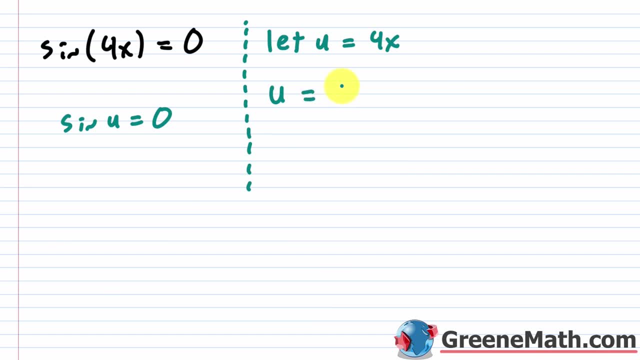 So let's come back up And let's say that u is equal to pi n. Now we let u be equal to 4x, So all I have to do is plug in a 4x for u, So 4x is equal to pi n, and then just solve for x. 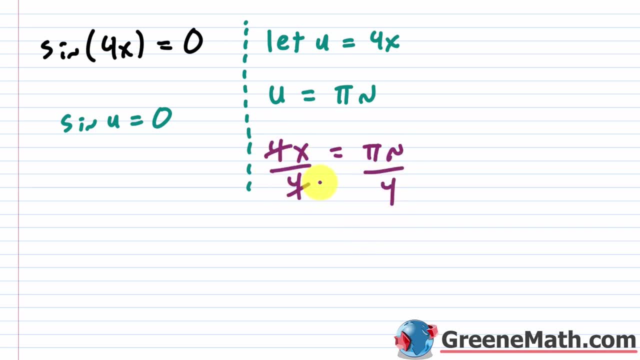 How do I do that? I divide both sides by 4.. So this would cancel and you're going to get that x is equal to pi over 4 times n. So let me get rid of this and bring this over here. So x is equal to pi over 4 times n. 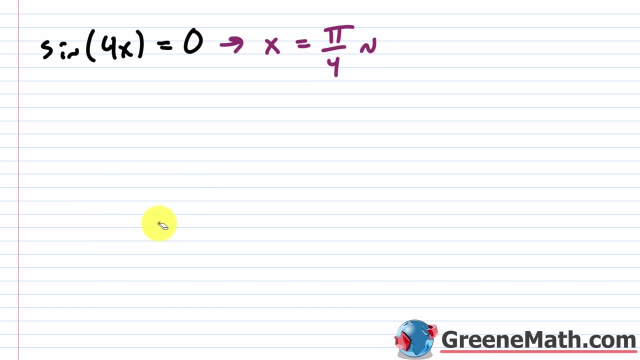 We will get our solution in the interval, in a moment. Let me get rid of this and let me come down here and solve this. So I'm going to use u again, but it's only in terms of this. It has nothing to do with what we did before. 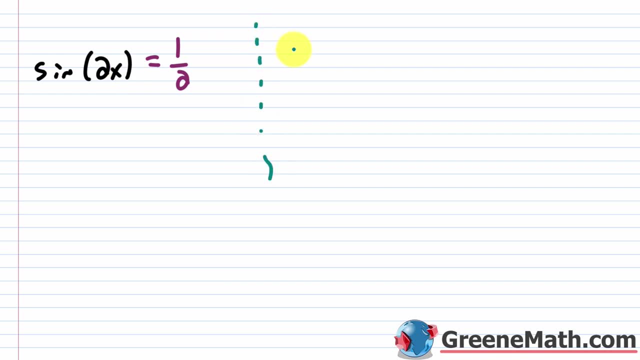 And actually, so nobody gets lost, Let me just pick something else. Let me let w- so nobody is confused- be equal to 2x. So now I want to solve: the sine of w is equal to one half. Come back to the unit circle and let's think about this again. 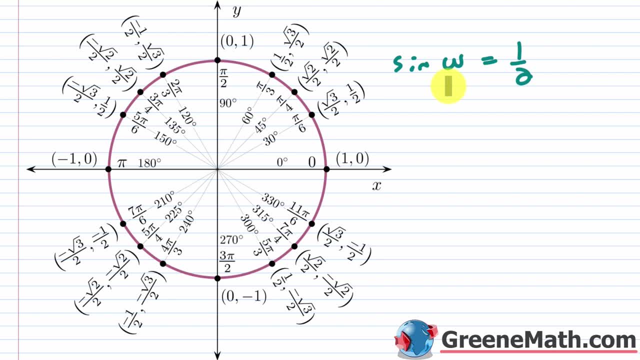 Sine of w equals one half. Well, we know how to solve that. We know that solutions are going to repeat every two pi. So where's the y coordinate? one half, So right here at pi over six, And then that's going to be right here at five pi over six. 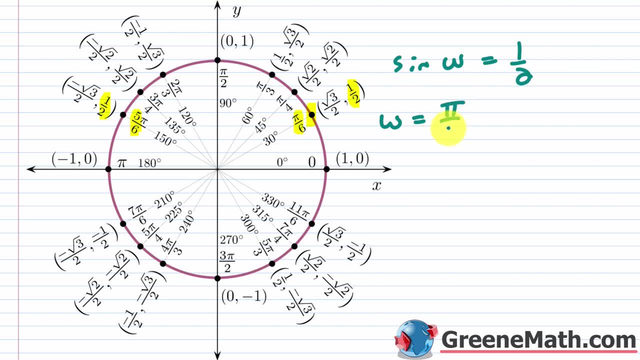 So we can say that w is equal to pi over six plus Again. these solutions repeat every two pi Again. this is in terms of w. So we're going to say two pi n and then we're going to have five pi over six plus two pi n. 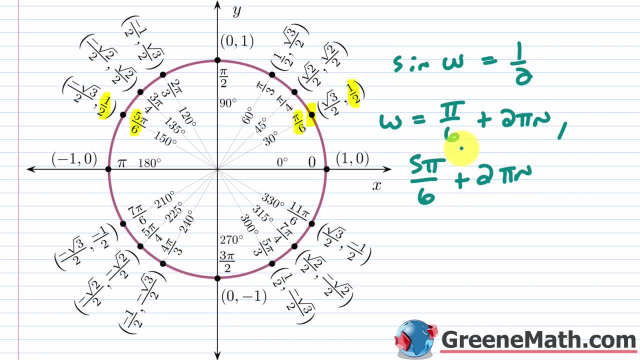 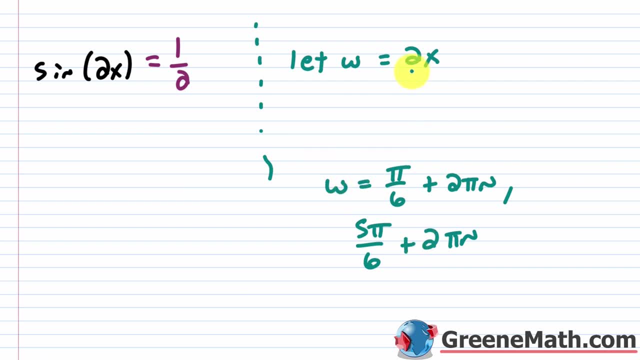 Again, things are happening. every two pi in terms of w. Okay, So in terms of w. So let's grab this, All right. So let's come back here, Let's get rid of this. And now w is two x. 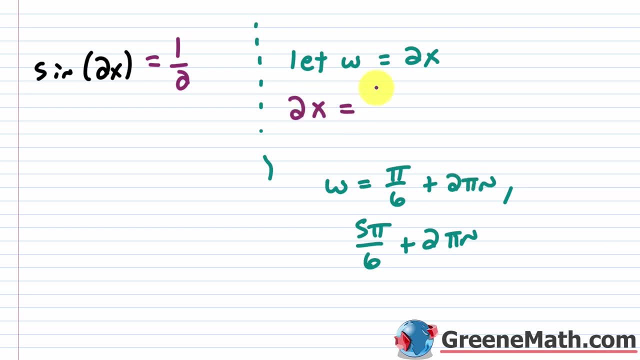 So all you have to do is go back and say: okay, well, two x is equal to: we have pi over six, and then plus you have two pi n. The other one is: two x is equal to five pi over six, plus two pi n. 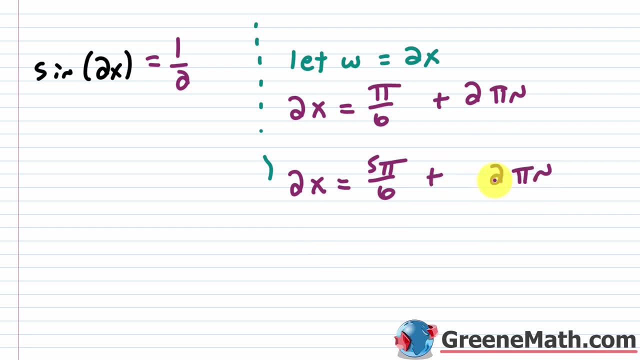 Let me get rid of this, And actually I probably should slide these over a little bit, because I have to do some multiplication here. Let me make that border a little bit better And let me slide this down just a little bit and slide this up just a little bit. 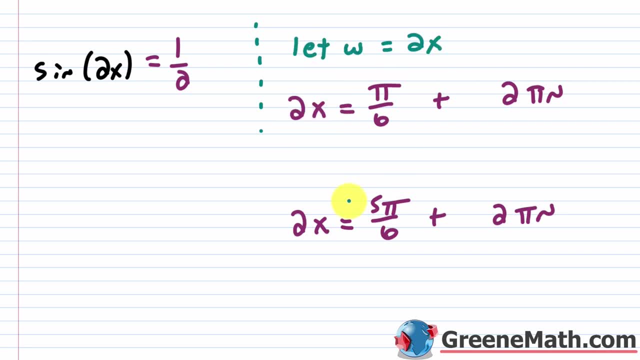 Now we have two x, not x. So if you want x by itself, you can divide everything by two, But because we have a fraction involved, it's better to multiply by half. It's just a little bit easier to do it that way. 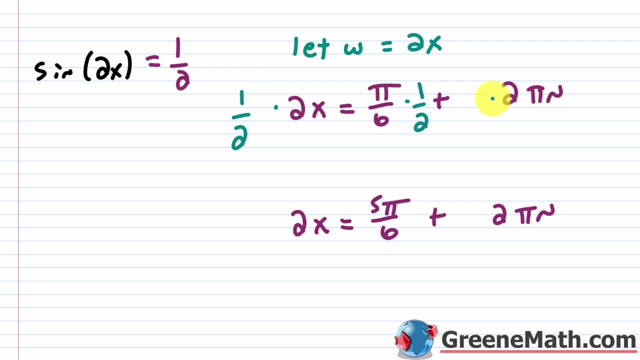 Let me get rid of this border here. So multiply by a half and then multiply by half, So we know that this would cancel. and just give me: x is equal to pi over six times a half, is pi over twelve, And then plus one half times two, pi n the twos would cancel. 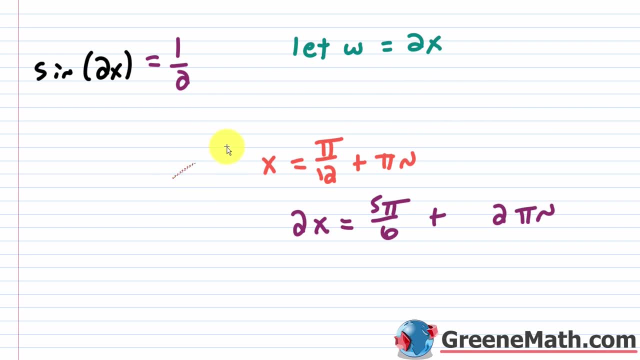 You just have pi n, So get rid of this. So that's one guy there. Let me move this over. And then this guy. I'm going to do the same thing, So let me move this up. I'm going to multiply this by one half. 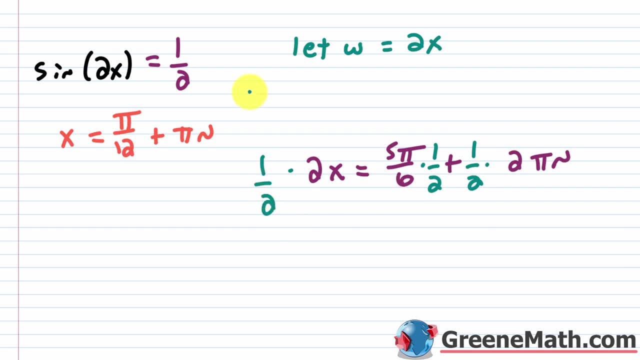 multiply this by one half and multiply this by one half. So we're going to see that the twos are going to cancel. You're going to have: x is equal to: if you have five pi over six times a half, Well, we would have five pi over twelve, and then plus again, the twos would 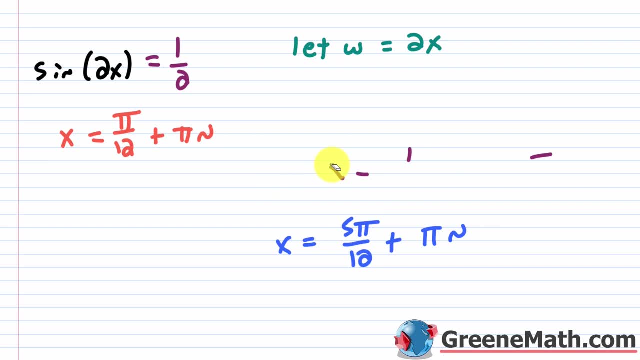 cancel, So you're going to get pi n, So let me get rid of this. And actually this color really doesn't show up very well, So let me change this and say that x is equal to pi over twelve plus pi n. 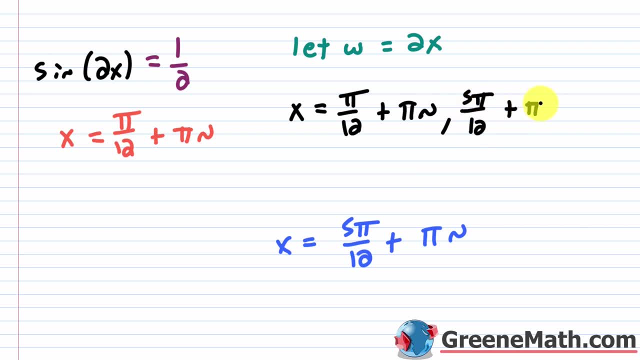 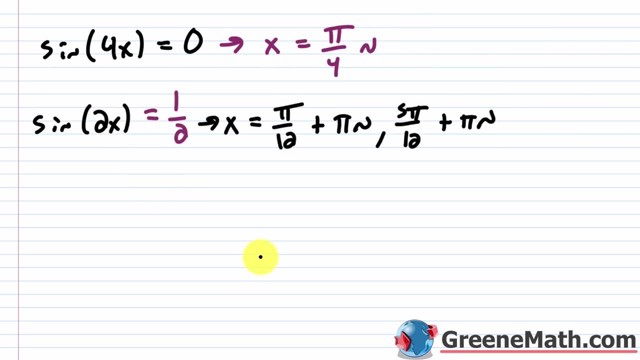 And then we have five pi over twelve plus pi n. OK, let me bring this back here and now. let's put our solution together. So right now I'm giving you the general solution and then I'll give you the solution over interval. So for the general, 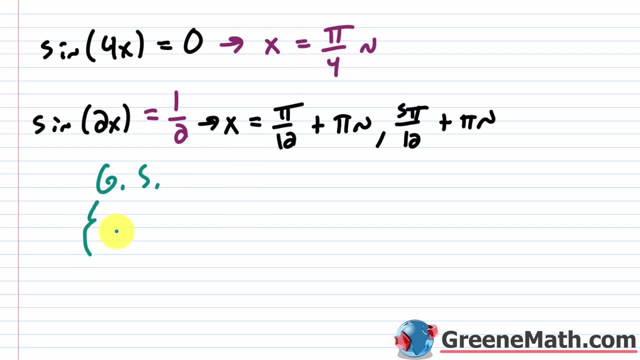 solution. you're going to take this one. So we're going to say that we have pi over four times n. Then, if we think about this one, we have pi over twelve plus pi n. And then this one is five pi over twelve plus pi n. 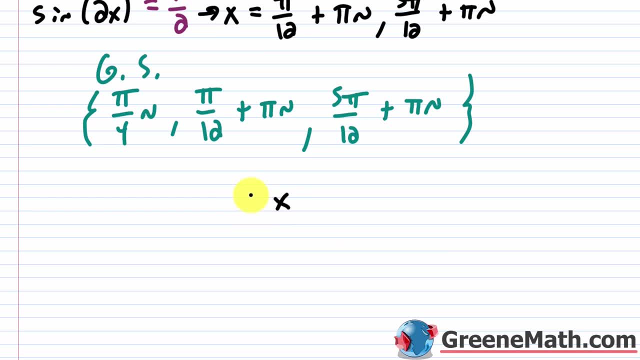 That's our general solution. Now, if we want to go with the solution where x is greater than or equal to zero and less than pi, Well, again, you're going to start here and plug in a zero for n, So that would give you. let's go. 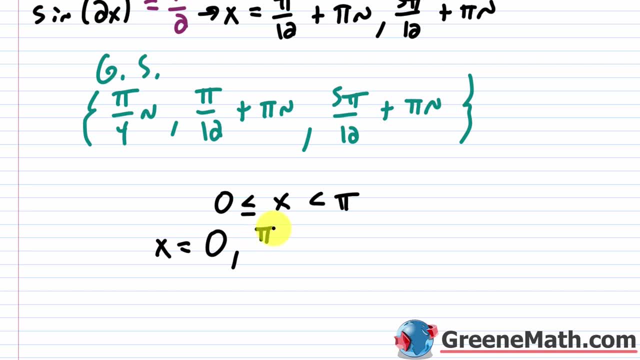 Let's say that x is equal to zero. And if I plugged in a one, I'd have pi over four. If I plugged in a two, I'd have two pi over four, which is pi over two. If I plugged in a three, I'd have three pi over four. 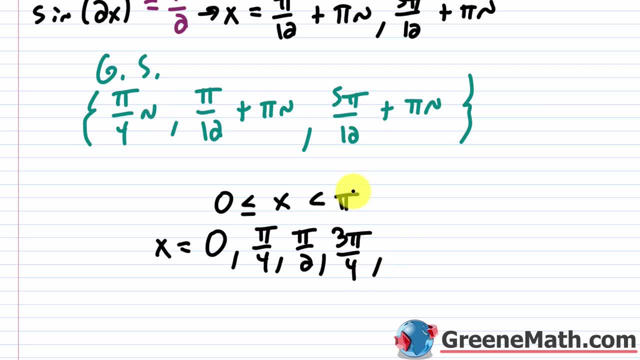 If I plugged in a four, I'd have four, pi over four, which is pi, and that's not in this interval. So I'm going to stop there. Then these: you would have pi over twelve if you plugged in a zero there And then if you add pi, you're not going to be in this interval. 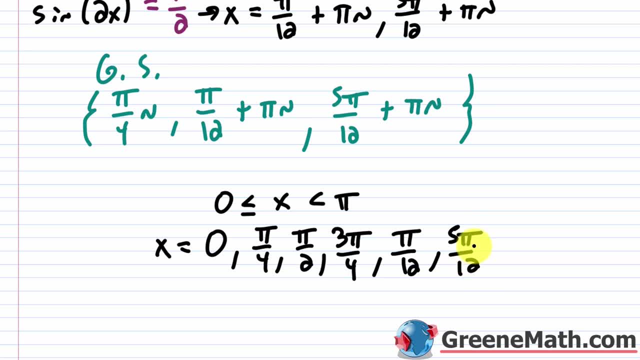 So then this one, I would have five pi over twelve. So five pi over twelve. Again, if I add pi, I'm not going to be in this interval. So these are your solutions in this interval. So zero pi over four, pi over two, three pi over four. 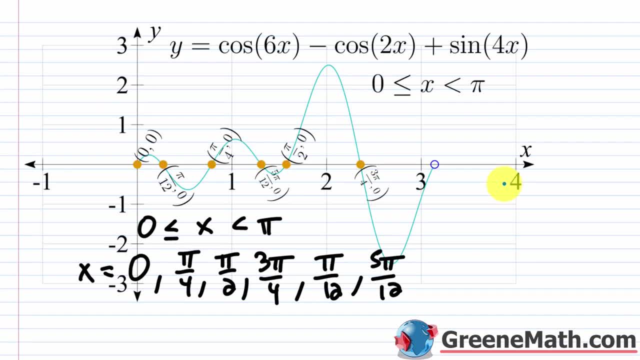 pi over twelve and then five pi over twelve. OK, so I want to think about this graphically with you. If you're struggling with finding the general solution, this can be extremely helpful, although it's extremely time consuming to think about this with a graph. 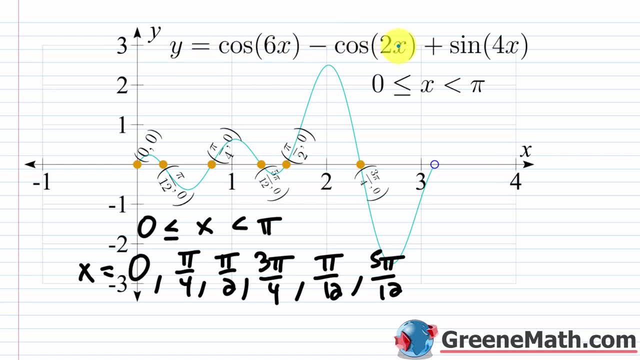 So we have: y equals the cosine of six x minus the cosine of two x, plus the sine of four x. So this was my equation. It's just that instead of y we had zero over here. So if I plugged in a zero for y, in other words 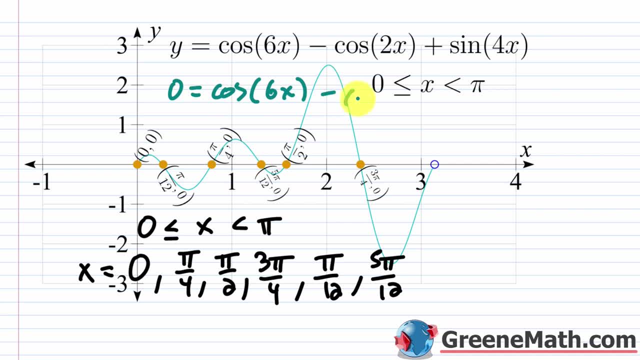 if I had zero is equal to the cosine of six x minus the cosine of two x plus the sine of four x. all I'm doing is I'm saying: for which x values am I going to get a y value of zero? Well, where is y zero when I'm thinking about this? on the coordinate plane. 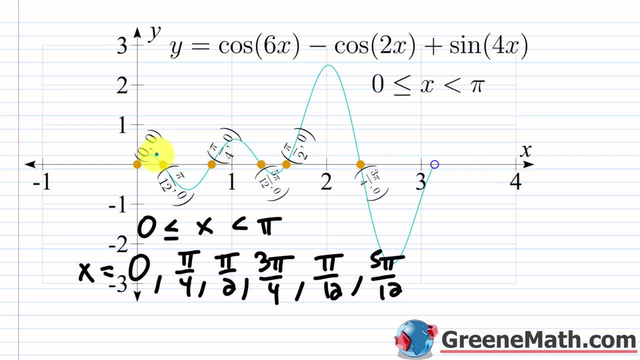 Well, that's on the x axis, right? So that's where y is zero. So anywhere where I cross the x axis or have an x intercept, I'm going to have a solution for this equation. So, thinking about this, where x is greater than or equal to zero, 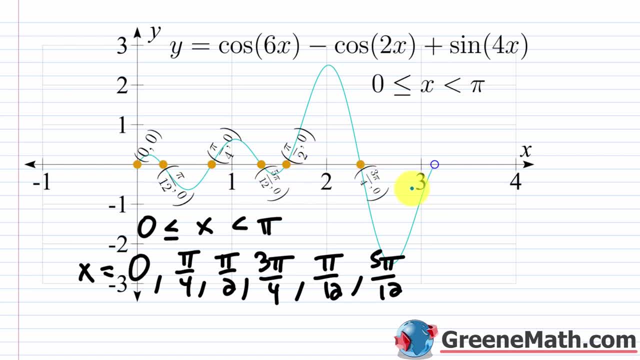 and less than pi. I get this graph right here Now. in a moment we're going to talk about the fact that the period for this guy is going to be pi. We discussed this in the last practice test. Maybe you didn't watch the video for that. 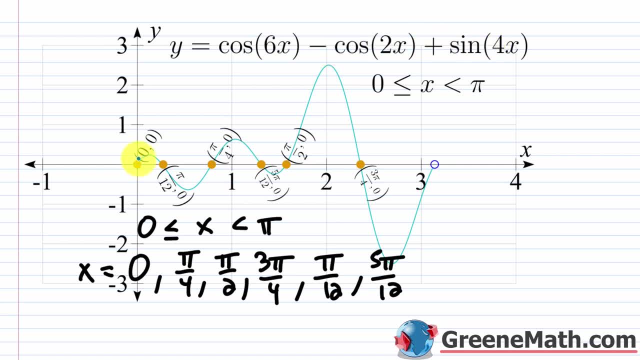 but I'll explain where this is coming from in a moment. So that means that I can go from zero to pi and I'm going to include zero and exclude pi and any solutions I find will actually repeat in that next cycle. So I could just take that solution and add pi. 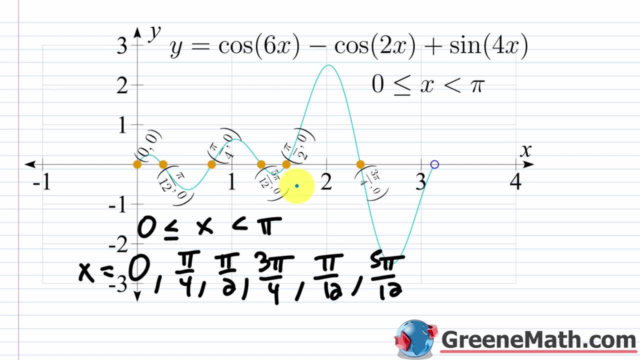 But you're going to see that you can condense some of those solutions that make it a little bit simpler, And let's just start with what we have. So notice that you have this zero here that matches this one. I'm going to skip this one over for a moment. 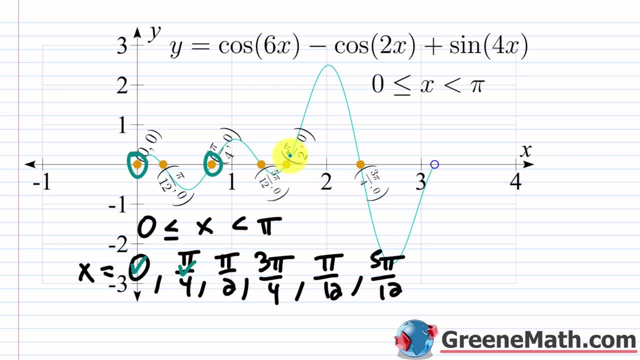 So we have this pi over four. That's there. I'm going to skip this one. So this is pi over two, So that's there, And then I'm going to go to this one, which is three pi over four. Now, if you think about those solutions, 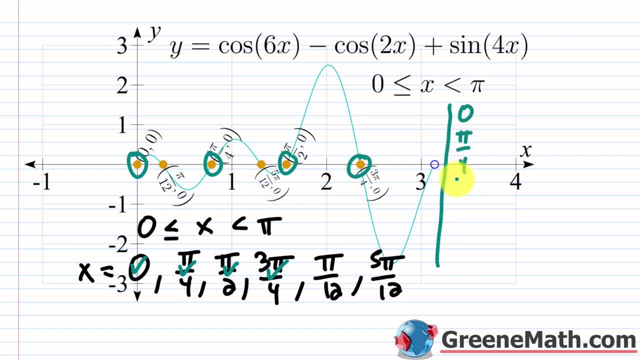 you have zero, and then you have pi over four, and then you have pi over two, And then you have three pi over four. Again. you could go through and say plus pi n and then plus pi n, and then plus pi n, and then plus pi n. 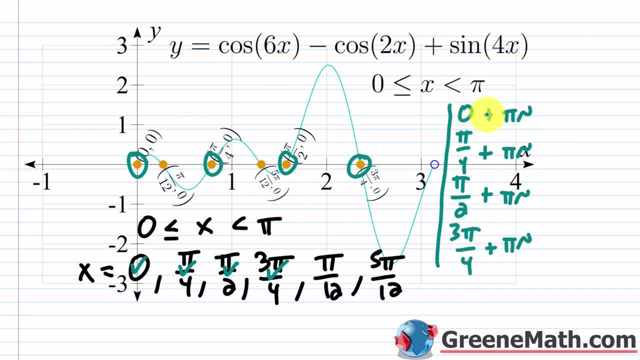 That is valid. But what's happening is if you add pi to this. Let me just show: if I added pi, this would get me to pi. If I added pi to this, I would be adding four pi over four. So this would get me to five pi over four. 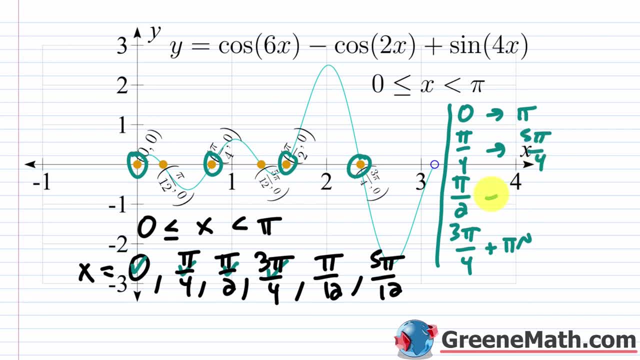 If I added pi to this, that would get me plus two pi over two, so that would be three pi over two. And then, if I added pi to this, I would add four pi over four, So that would get me to seven pi over four. 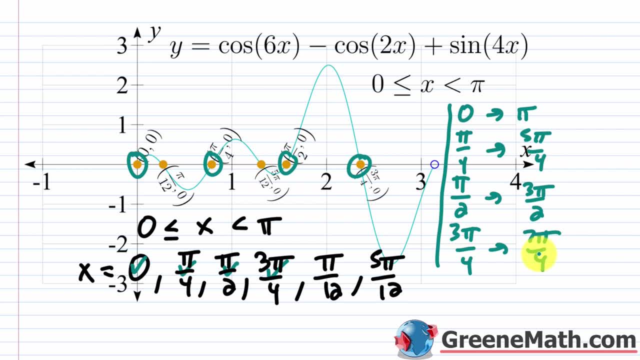 Well, if you go through here and you just look at these first guys here, so it would be a jump of pi over four each time. So zero plus pi over four is pi over four. Pi over four plus pi over four is pi over two. 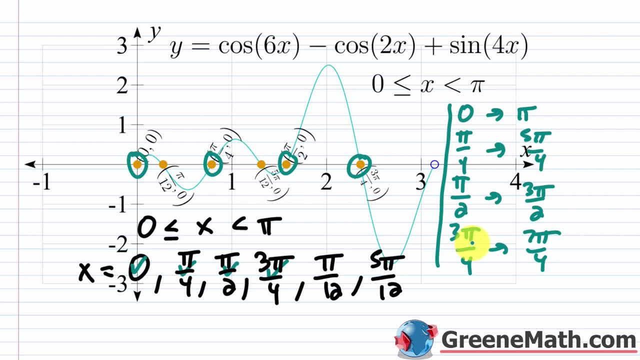 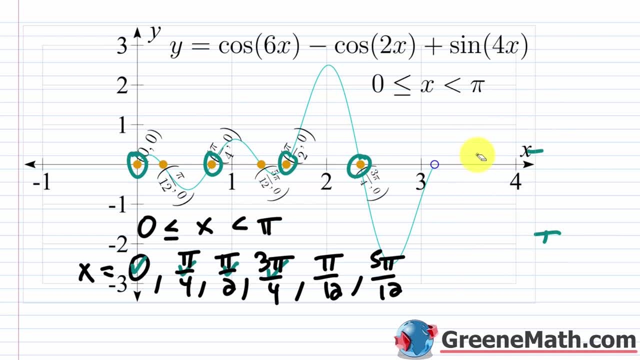 and so on and so forth. So that's why we got that pi over four times n with the general solution. So we have this pi over four times n. Then the other ones. you really can't do anything with them other than to say that you have pi over 12.. 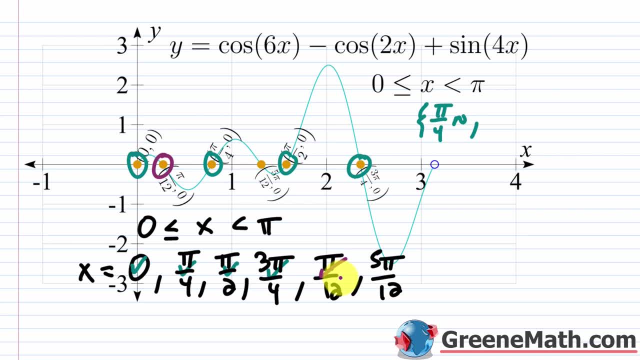 So that's this one right here, and then just plus pi n. So it's just going to repeat in the next cycle. So this is pi over 12 plus pi n. Let me slide this down And then the other one. we have five pi over 12.. 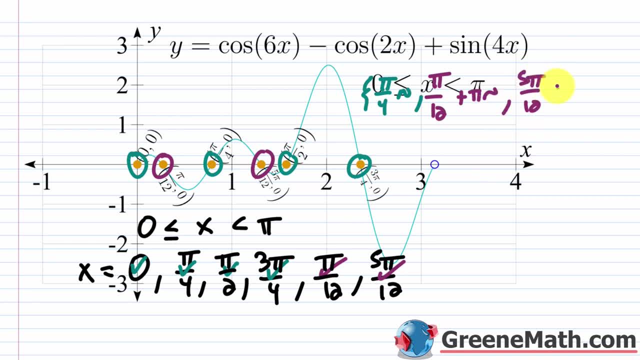 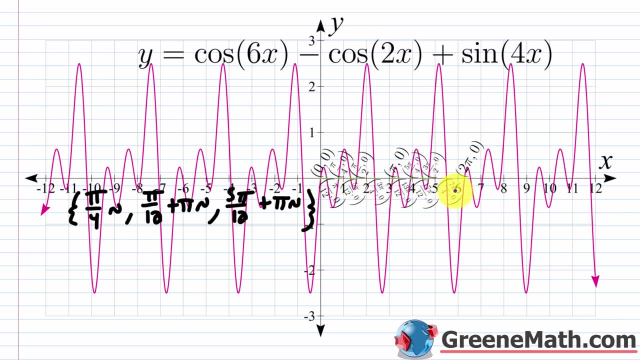 So that's this here. So again, that's just gonna repeat in the next cycle. So five pi over 12 plus pi n. All right, let's come to the graph Now. these solutions are extremely hard to read, So you probably need to follow me on Desmos. 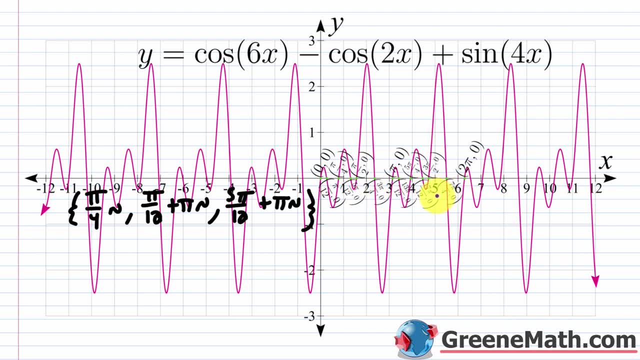 or something like that, in order to fully see everything. But I'm just gonna first talk about the period for this guy. I'm gonna let you visually see that and explain where it's coming from. So in the practice tests for the last lesson: 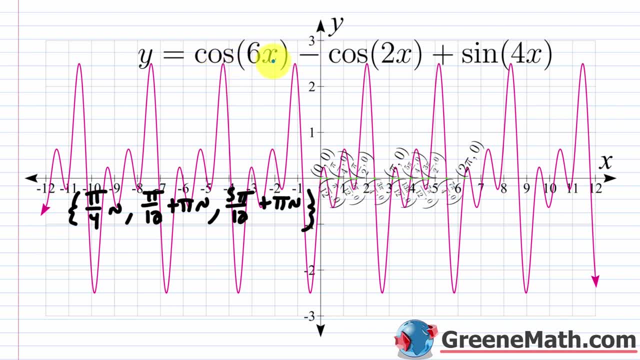 we talked about the fact that if you had something like, y equals the cosine of six x minus the cosine of two x plus the sine of four x. if you wanted the period for this, then basically you would have to do this. Basically, you would think about: 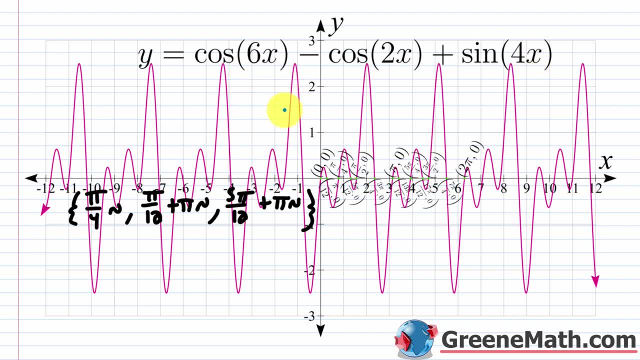 the least common multiple of the periods. So how do you get the least common multiple of the periods? So this right here, you'd think about it as, let's just say you had y equals the cosine of six x. What's the period? 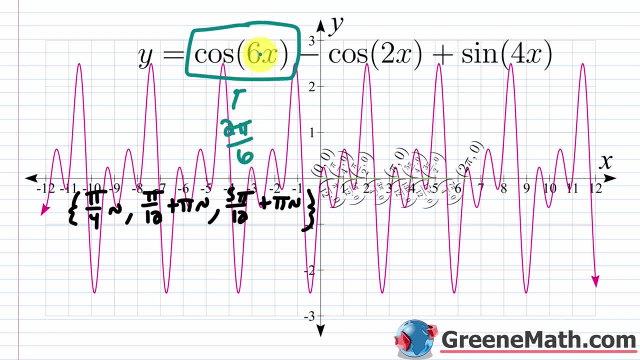 Well, it's going to be two pi over six, right, Two pi over six, which is pi over three. So pi over three Again. that's coming from that formula. If you have, y is equal to the cosine of bx. 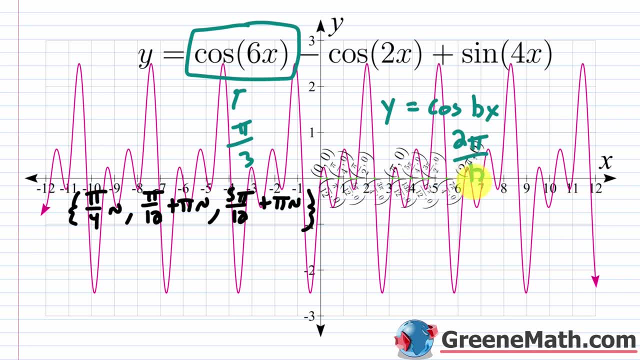 well, it's two pi, which is the standard period for cosine, divided by b. So here it's two pi divided by six. That gives me pi over three. It's the same thing if you run into sine right. So sine and cosine is the same thing. 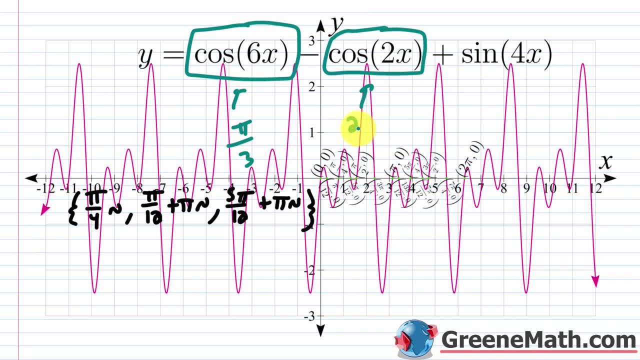 So let's do this one. So this is the cosine of two x, So that's two pi over two. So that gives me just pi. And then for this one it's the sine of four x, So that's two pi over four. 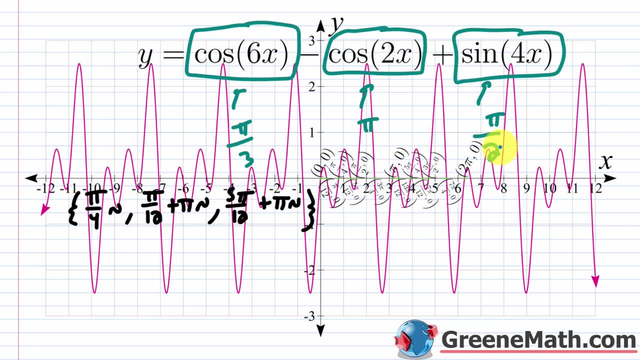 So that's pi over two. So we have not discussed how to find the least common multiple of fractions. So, in other words, let's say I said what is the least common multiple of one third, one and one half? Well, some of you know that it's going to be one. 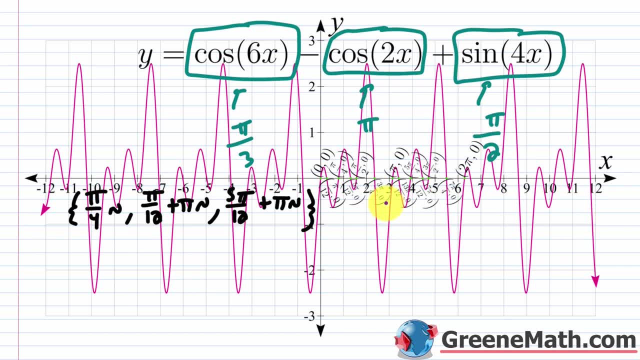 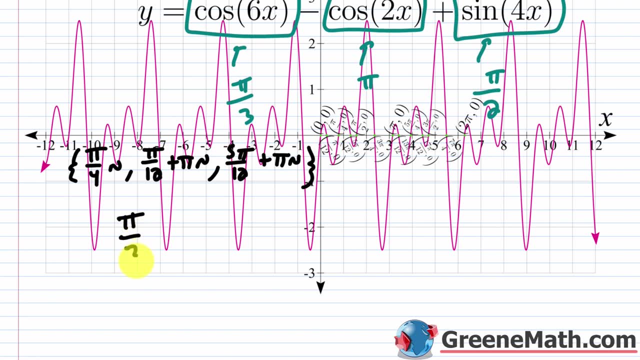 but others don't. Now there's a formula You can use for it, but it's a little bit complicated. actually, If you ask me, I think it's a little bit faster to just list things. So if you had something like pi over three, 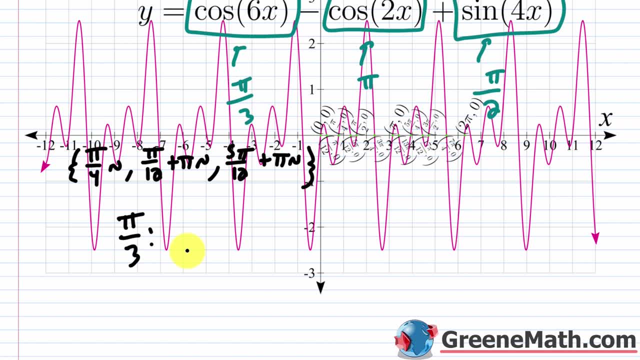 all you're doing is you're multiplying it by one, then two, then three, then four. You're generating some multiples. So times one, it would just be pi over three, And then, times two, it would be two, pi over three. 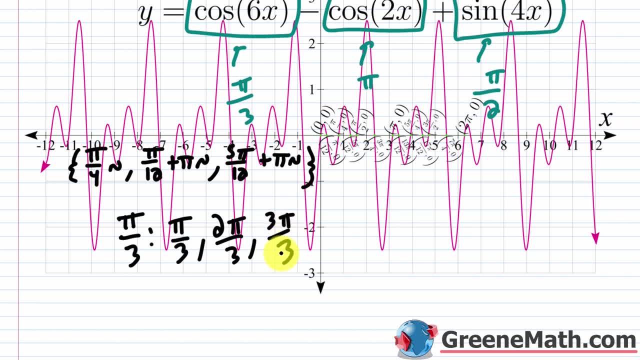 And then times three, it would be three pi over three, which of course is just pi, And then we could just do one more. So times four would be four pi over three. Let me put a border For this one, if it's pi. 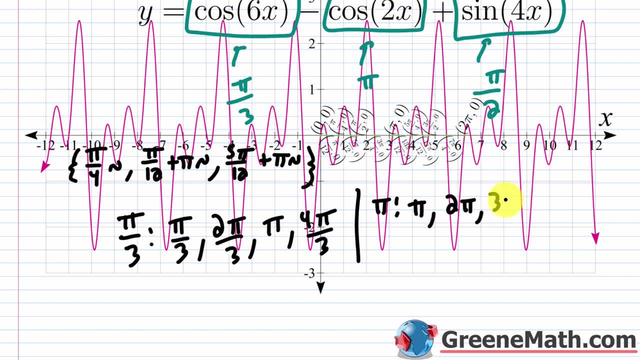 well, that's real easy. Multiply by one, you get pi, then two pi, then three pi. Let's stop at four pi, Then for the other one you have pi over two. So let's go times one, it's pi over two. 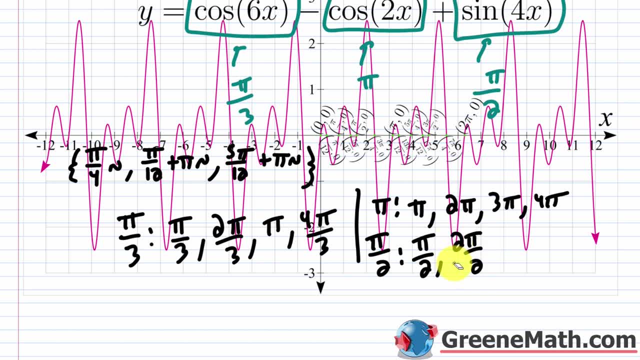 Times two, it's two pi over two, which of course is going to just be pi. And then times three, it's three pi over two. Times four, it's going to be two pi. And you could stop there If you look at the least common multiple here. 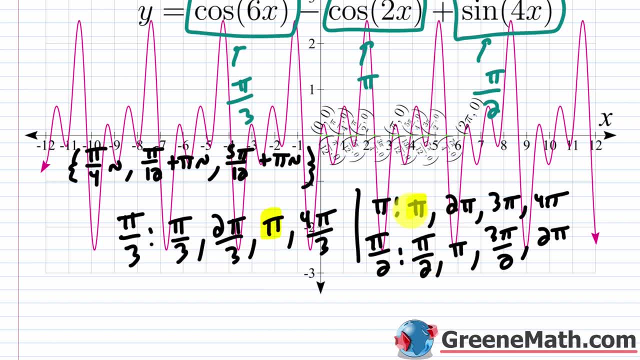 well, looking through, what do I have? that's common to everything: You have pi, you have pi and you have pi. So, in other words, if you had one, if you had one and you had one, half the LCM would be one. 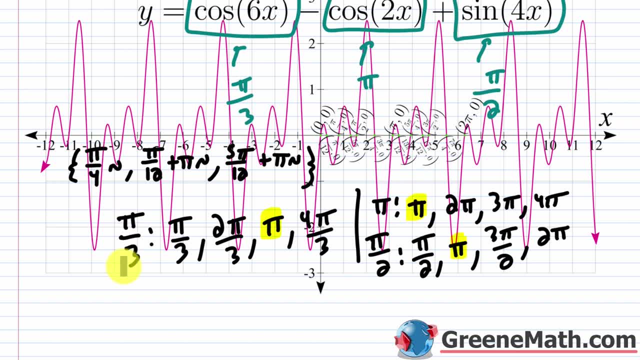 But in this case we have pi over three, which can be thought of as one third times pi. You have pi which can be thought of as one pi, And then pi over two, which you could think of as one half times pi. 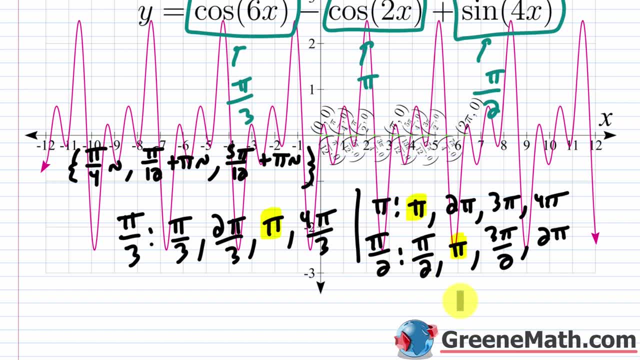 So the least common multiple there is pi. So that tells me that the period for this graph here is going to be pi. Let me get rid of this And let me actually trace this out so you can see it If you want to follow me. 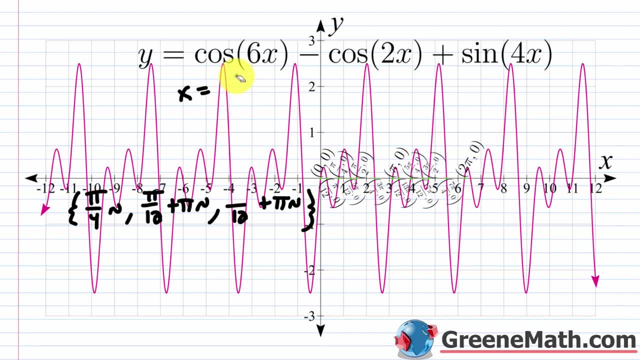 type in x is equal to pi like this in Desmos. It's going to fix it for you and give you a pi like that You're going to get. you're going to get a vertical line. You can go. x equals two pi. 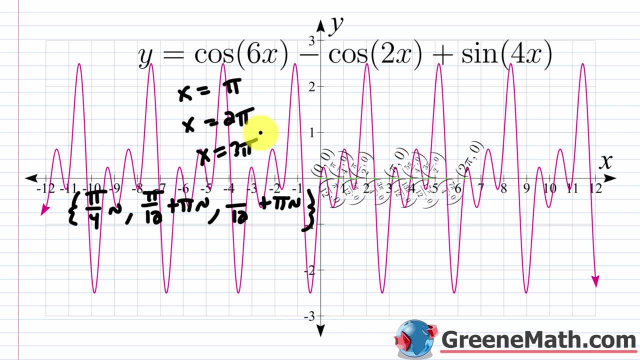 and then x equals three pi, so on and so forth. You're going to get these vertical lines and it's going to really allow you to see the period of this guy. So I'm just going to trace from zero to pi And then we'll see that this is going to repeat. 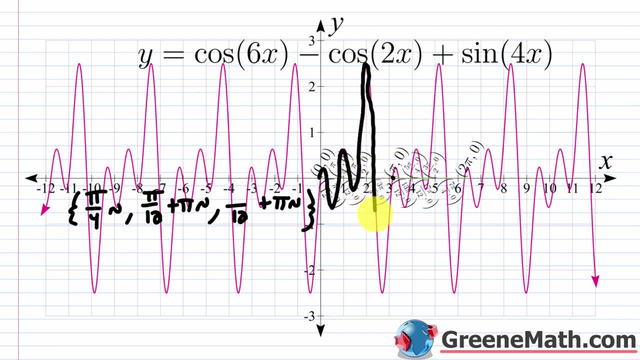 from pi to two pi. So this right here, this is going to be one cycle for this graph. So this is one cycle. So from zero to pi, And then again, if I went from pi to two pi, the same thing is going to repeat. 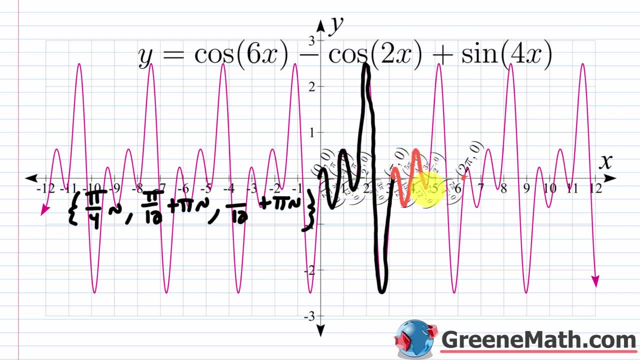 So if I went from pi to two pi, So basically I come up, come down, come back up, come down, come back up. So this is way up here. This is exactly matching what happened in the last cycle, So you can see that these two match. 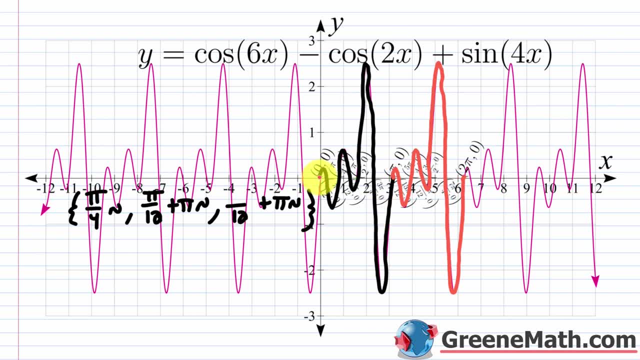 and the period is going to be pi. So this tells me that things that happen from zero to pi- zero included, pi excluded- would happen again from pi to two pi- pi included, two pi excluded. So that's how we ended up on the last page. 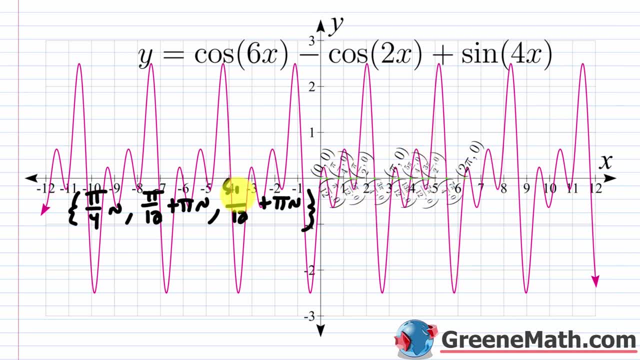 where I did this, where you could see the solutions more clearly, And it looks like I erased my five pi over 12.. But, as I was saying, it just shows you that solutions that happen in this cycle will repeat in the next cycle. 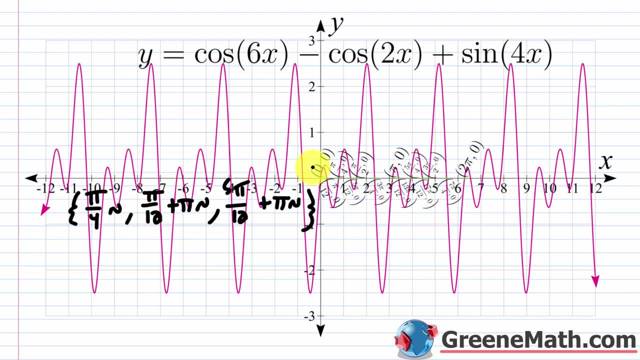 So you can take your zero plus pi? n. You could take your pi over 12 plus pi n. You could take your pi over four plus pi n, so on and so forth. It's just that the zero pi over four, pi over two. 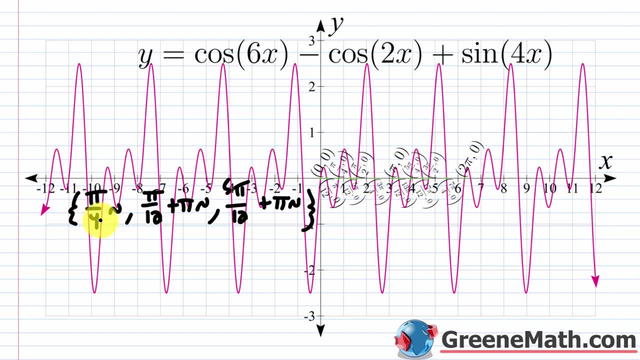 three, pi over four. those guys can be condensed into this form right here, So the pi over four times n, where n is any integer. And then for your pi over 12,. well, you really can't do any better than just saying: plus pi n. 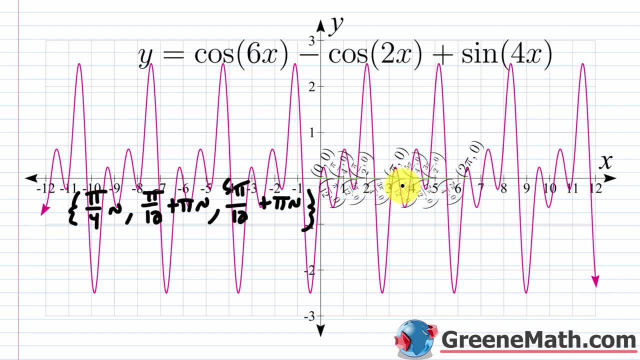 So you have your pi over 12,. you add pi. that gets you to that 13 pi over 12.. I know you can't see it, but it's right there. And then five pi over 12, again, if you add pi. 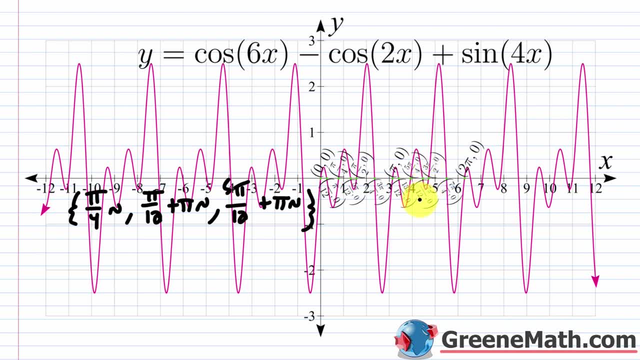 you're going to be at that 17 pi over 12.. Again, I know it's hard to see, but just follow it on Desmos if you want to look at it. So this is our general solution. Again, if you want to play around, 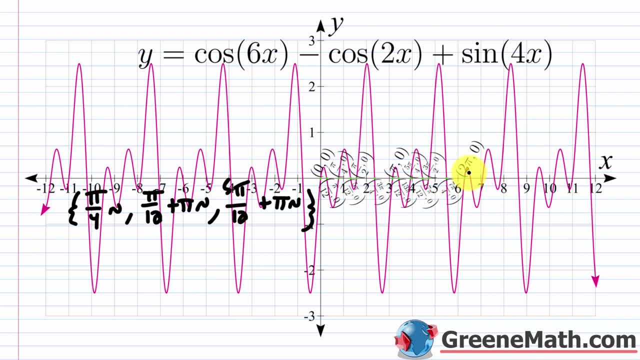 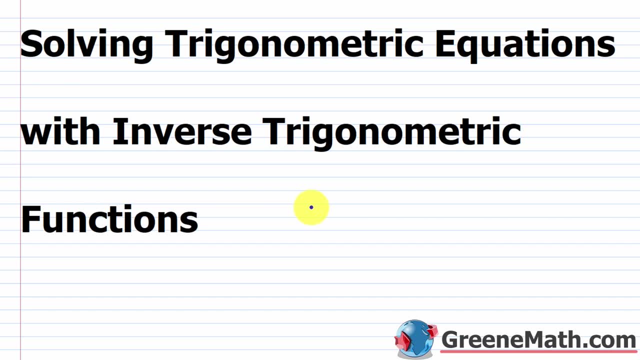 with the graph on Desmos, you can visually see this and it'll help you to understand the concept of the general solution and how things are repeating. In this lesson we want to talk about solving trigonometric equations with inverse trigonometric functions. 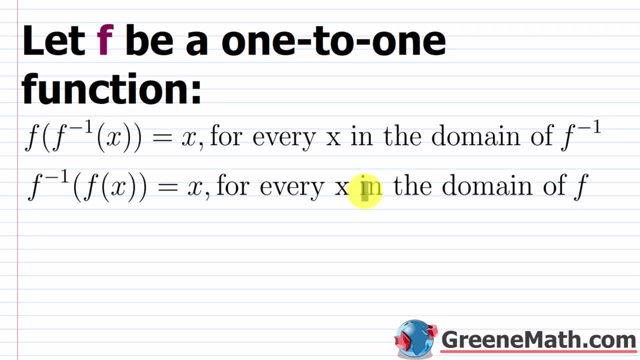 All right, before we start looking at any equations, I want to review some concepts that are going to be important for today's lesson. So these are going to come from our lesson on inverse trigonometric functions, So I'm going to let f 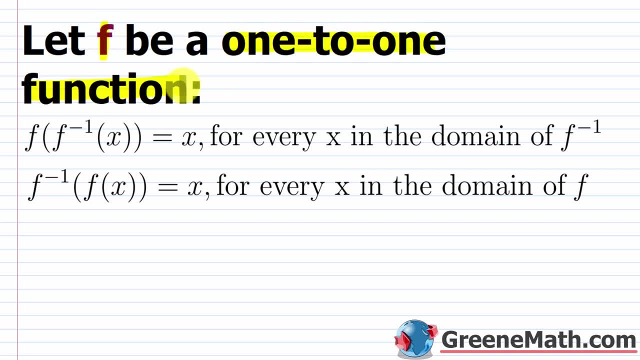 be a one-to-one function. What does it mean to have a one-to-one function? Again, if you go back to the definition of a function, you have a relation where for each x there's one y. So you would look at the graph. 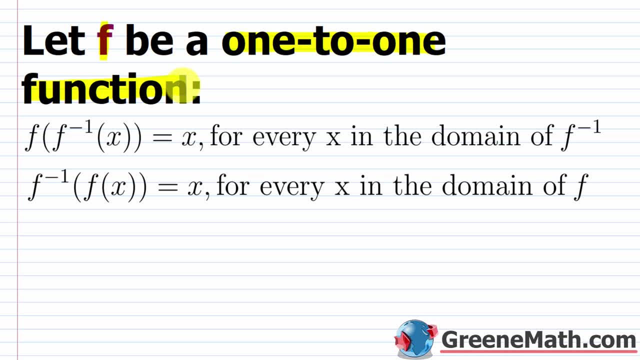 of the relation and it needs to pass the vertical line test. So no vertical line would impact the graph in more than one location. And if it passes that, you have a function. So for each x there's one y. Now, when you think about: 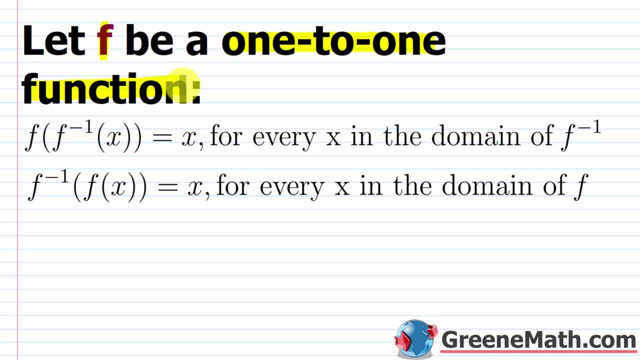 a one-to-one function. you start with a function and you apply another rule where you say: now also for each y there's one x, So for that you would check it with the horizontal line test. So no horizontal line would impact the graph. 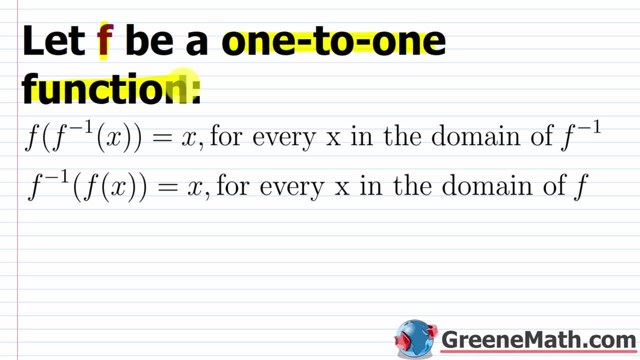 of a one-to-one function in more than one location. If it does, that's not a one-to-one function. If it doesn't, then you're good to go and you have a one-to-one function. And if you have a one-to-one function, 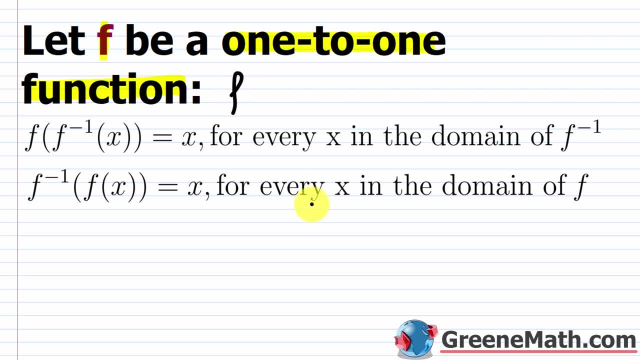 you can generate an inverse. So let's say f is your one-to-one function. The way you would notate your inverse, you would say it was f inverse, like this. So again, this is not an exponent of negative one. This is the inverse of my function, f. 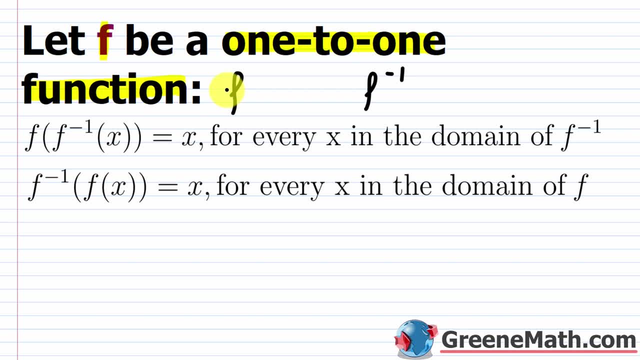 The way you generate your inverse is you swap your x's and your y's, So the domain or the set of allowable x values for f becomes the range or the set of allowable y values for f inverse, And then the range for f becomes the domain for f inverse. 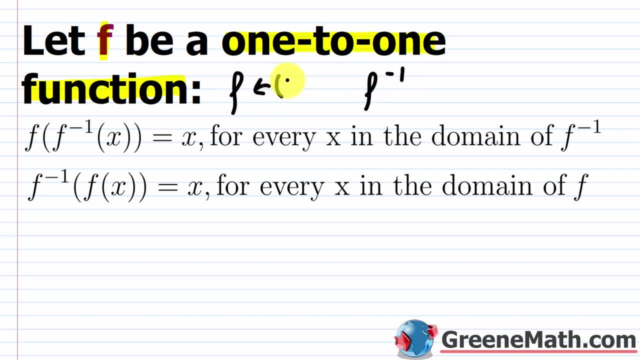 So, in other words, if I look at a point on f, and let's say it's three comma two, when I go to the inverse, these guys are going to be swapped. So the x will become the y and the y will become the x. 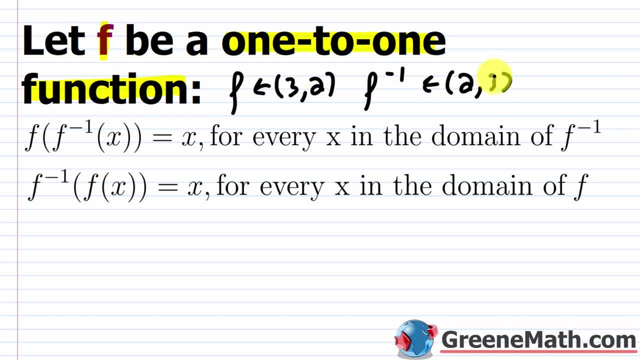 So this would be two comma three. So your x value of three becomes your y value of three- and that could be a lot better there- And then your y value of two will become your x value of two in the inverse. So, following this thought process here, 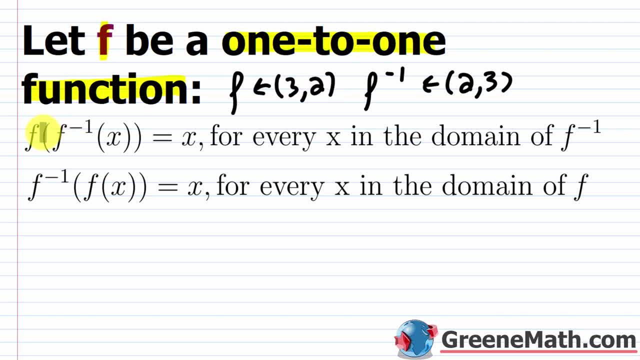 where the domain becomes the range and the range becomes the domain. what happens is when you look at your function and you compose it with its inverse, you're going to have this little cancellation. that happens where you can say: these guys are going to undo each other. 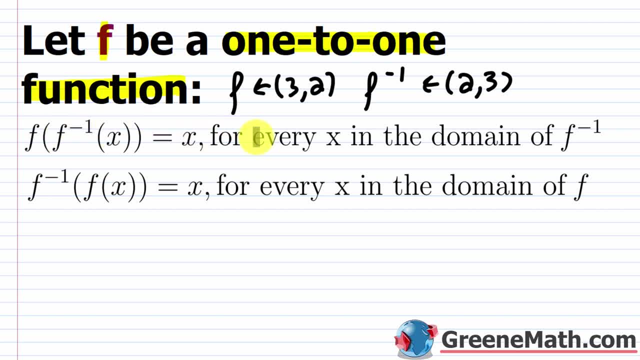 So f of f inverse of x is equal to x for every x in the domain of f inverse. And then f inverse of f of x is equal to x for every x in the domain of f. So this is something we're going to use today. 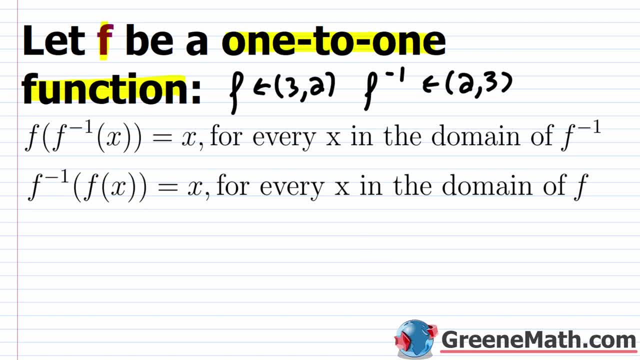 when we're solving our trigonometric equations. So as a practical example, just using what we have here, let's say you had f of f, inverse of, let's say, two. So using this right here, it should be equal to two. 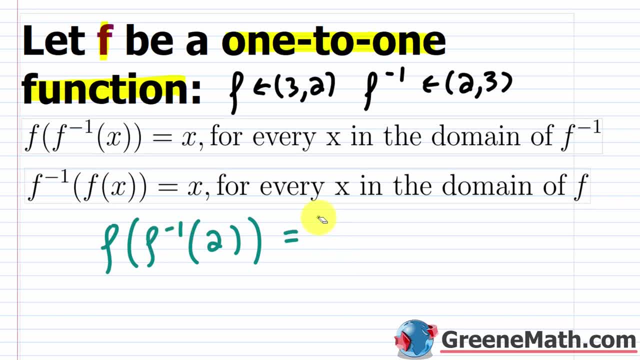 So I can just give an answer of two right away. But if you wanted to prove this, you can go about it the long way. So you could say: what is f inverse of two? Well, I come up here and I say: 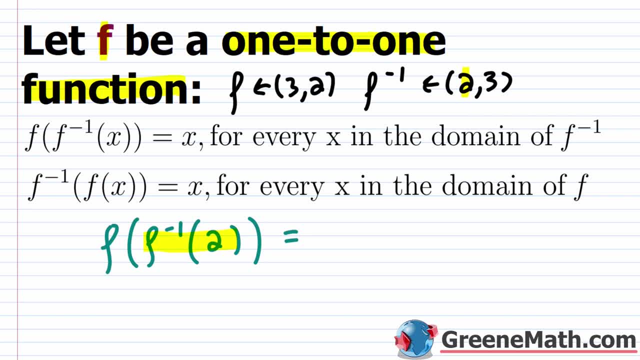 okay, here's an x value of two. If I plug that in, I know that my output, or my y value, is going to be three. So what I want to do is say that this is now f of three. Okay, well, what is f of three? 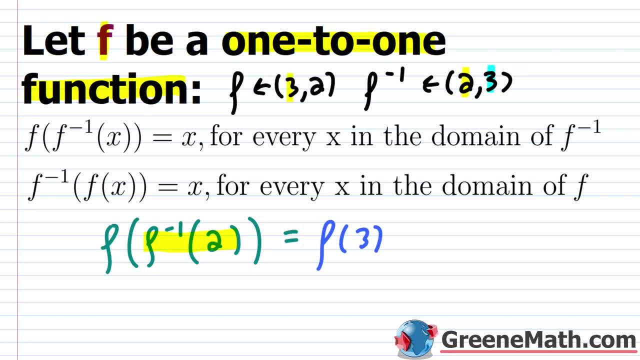 Well, again, if I look at my x value of three, the associated y value is going to be two now. So this is going to be two. So again, f of f, inverse of two, is going to give me two at the end of the day. 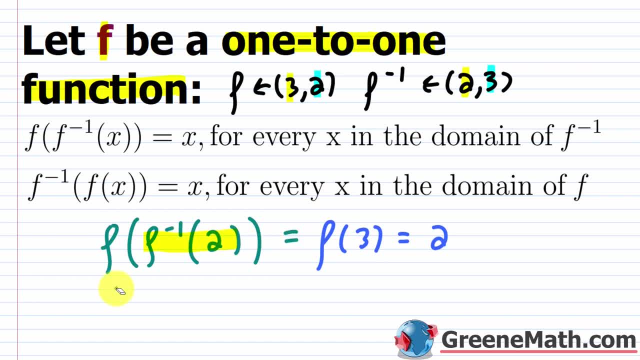 I can shortcut this and not go through this inside part Now when I look at the other one. in that case we have f inverse of, let's say, f of three. Well, again, I already know that this is going to give me three. 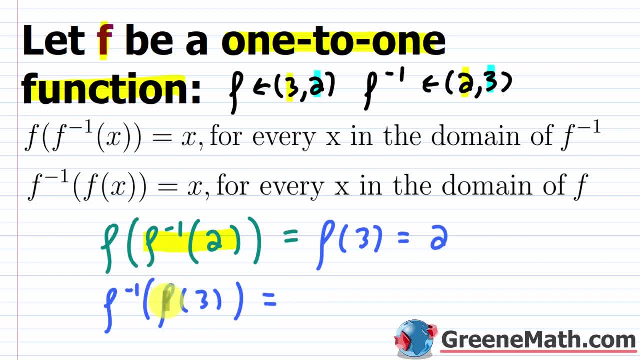 If I go about this the long way again, if I start on the inside of this guy right here, well, what is f of three? f of three is two. So this would be f inverse of two, and f inverse of two is going to be three. 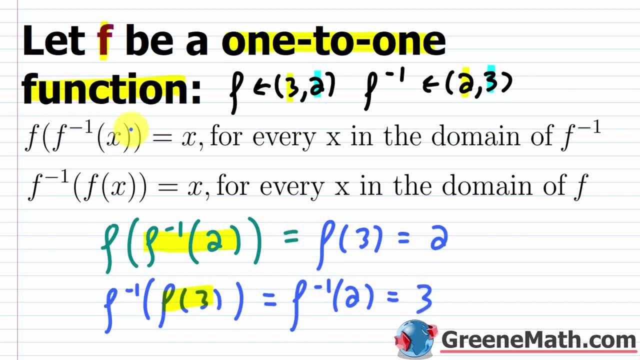 So these guys are just undoing each other. Again, f of f inverse of x is equal to x As long as x is in the domain of f inverse. and then f inverse of f of x is equal to x, Again, as long as x is in the domain of f. 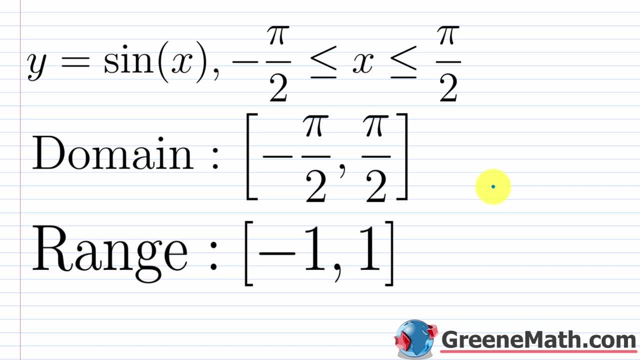 All right, let's continue reviewing our lesson on inverse trigonometric functions. So if we look at the graph of y equals the sine of x, we can see the domain is from negative infinity to positive infinity and the range is from negative one. 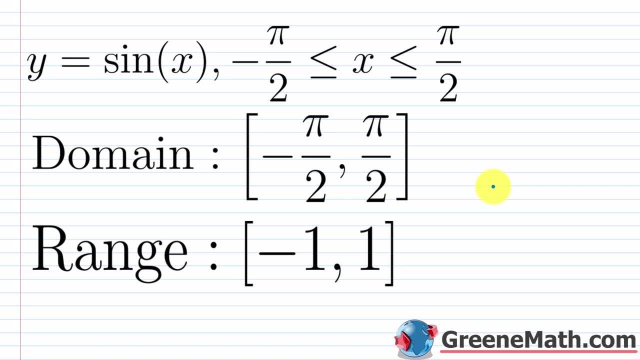 to positive one, with both being included. We can also see that it's not a one-to-one function. It would fail the horizontal line test. So if we want to find the inverse sine function, we can't start with just: y equals the sine of x. 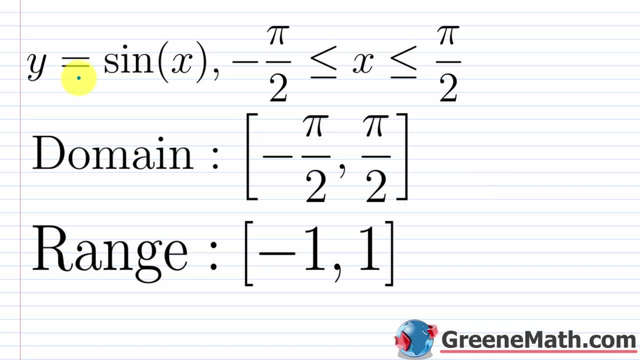 We have to do something called imposing a domain restriction, and we're going to come up with this, what we call restricted sine function. So y equals the sine of x, where x is going to be greater than or equal to negative pi over two. 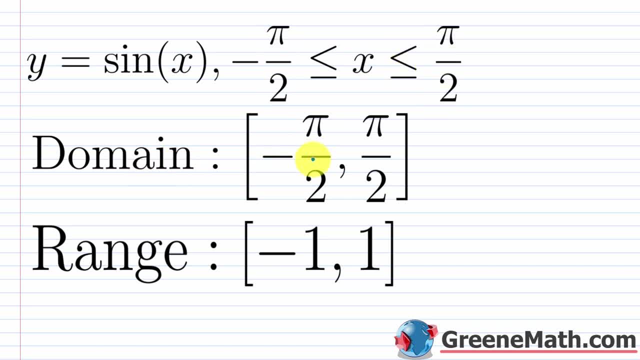 and less than or equal to pi over two. So I have this listed as the domain from negative pi over two to pi over two, with both being included. So when you restrict the domain, you end up with a one-to-one function with the same range. 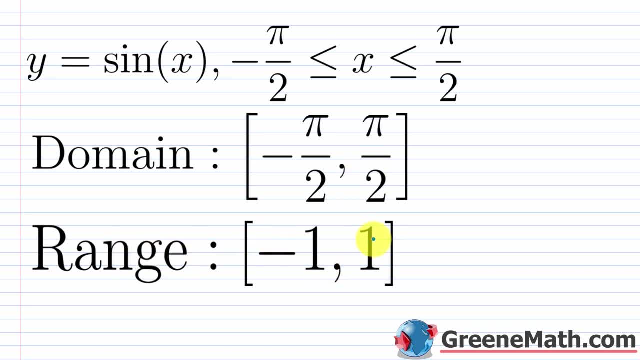 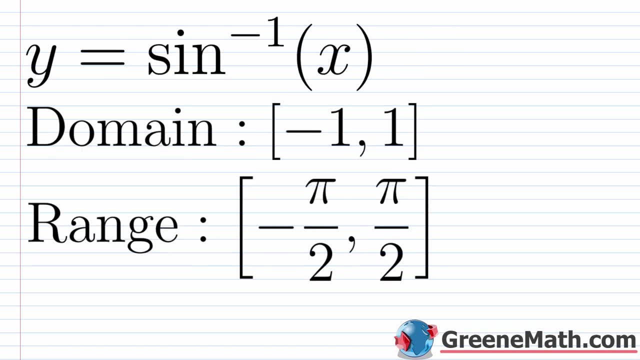 So the range is still the same from negative one to positive one, with both being included. When you start with a restricted sine function and you swap the x's and the y's, you're going to generate your inverse sine function. So y equals the inverse sine of x. 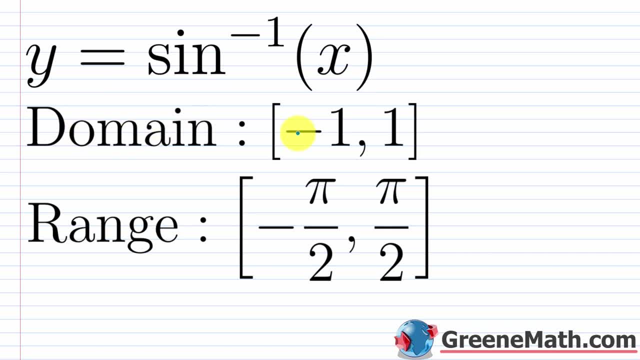 So you could say: y equals the arc sine of x. And now the domain which is from negative one to positive one, both being included, is coming from the range of your restricted sine function, And then the range from negative pi over two to pi over two. 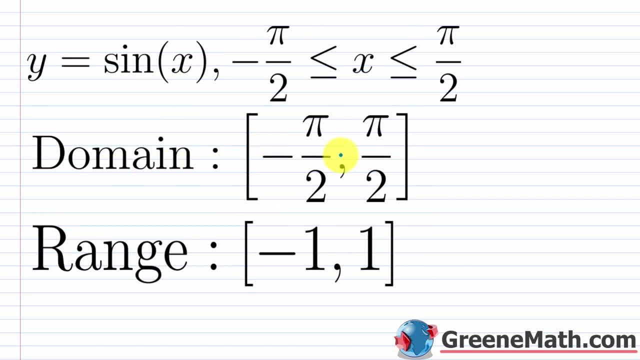 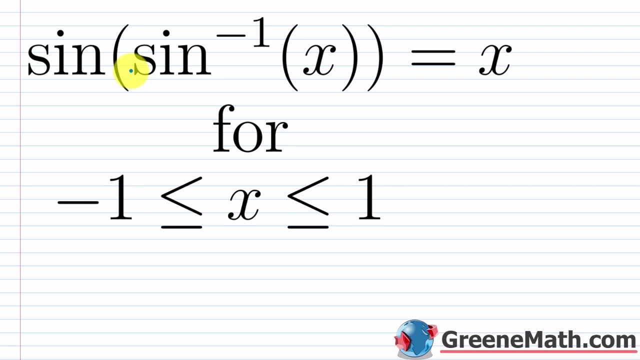 again, both being included is coming from your domain of the restricted sine function. Now the reason. it's important to know all that when you start using the cancellation properties with sine. you need to understand when you're going to do this. you need to know. 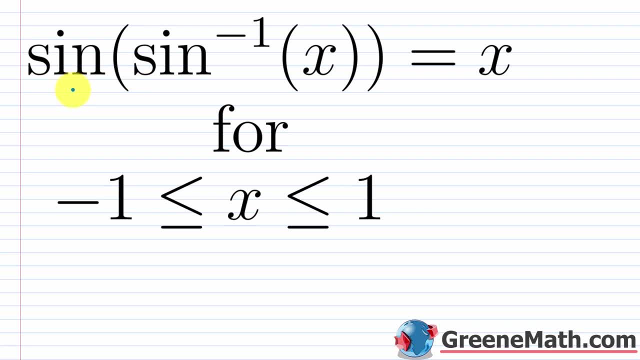 when you're composing sine with this inverse, when are you going to be able to cancel things? So, in other words, we like to cancel this with this and say, okay, well, the result of this is just going to be equal to x. 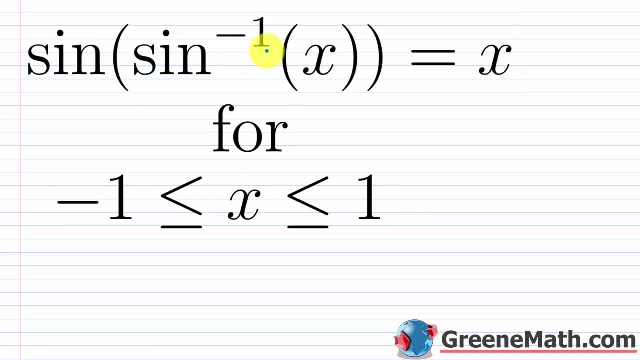 But this is only true if x is in the domain of the inverse sine function. And the domain of the inverse sine function is from negative one to positive one, with both being included. So the sine of the inverse sine of x is equal to x, for x being greater. 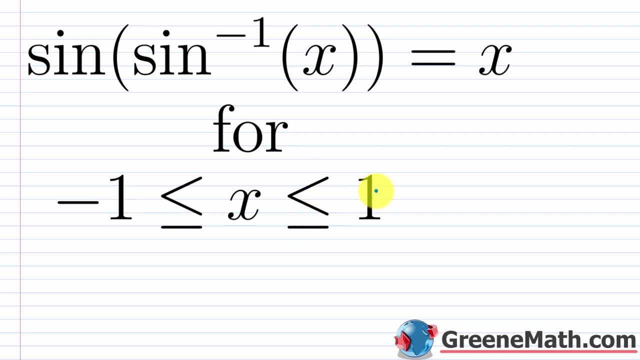 than or equal to negative one and less than or equal to positive one. If you pull out your calculator and you try to do sine of x of the inverse sine of two, that is not going to give you two as a result, It's going to give you an error. 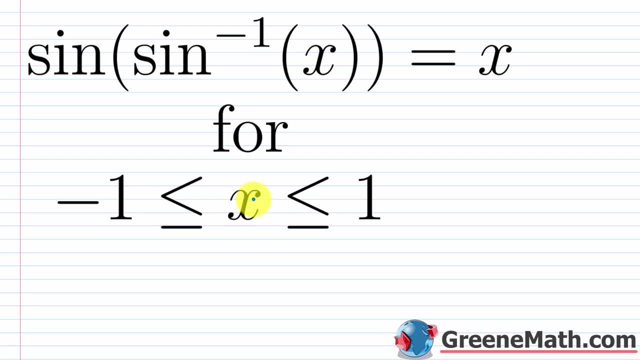 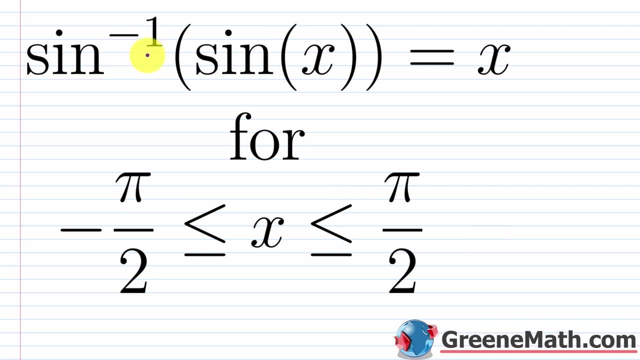 because two is not in the domain of the inverse sine function. All right, the next one is a little bit more challenging to understand. You can explain it with two different approaches. So if you have something like the inverse sine of the sine of x, 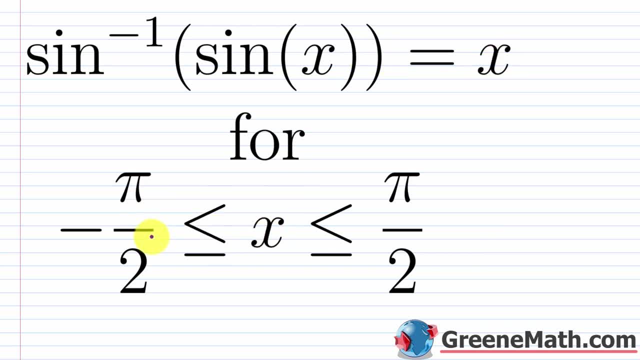 is equal to x. this is only valid for x being greater than or equal to negative pi over two and less than or equal to pi over two. So this is actually pretty important to understand. The first way to think about it is: let's say: you look. 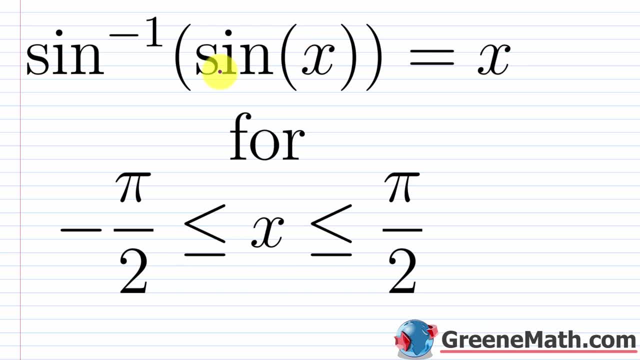 at the sine of x. that is not the restricted sine function. So we know that for this guy the domain is all real numbers and plugging something in from negative infinity to positive infinity is going to give you a result that's going to be from negative one to positive one. 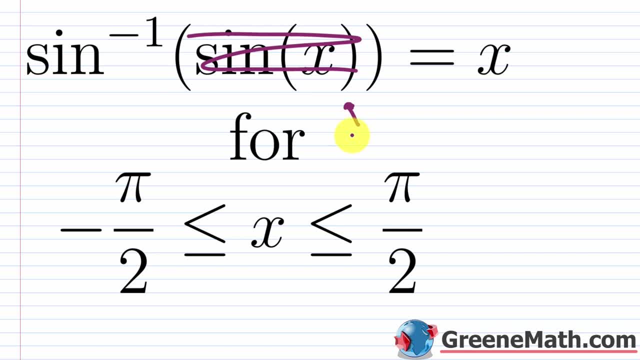 So I'm just going to mark that out and say that what's going to be plugged in for the inverse sine function is going to be from negative one to positive one. Well, you know that that's the domain for the inverse sine function And I know that the range 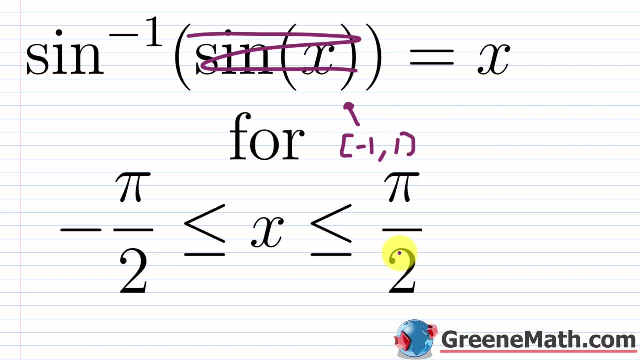 is going to be from negative pi over two to pi over two. So basically I'm always going to get something out of this guy right here. that's from negative pi over two to pi over two. But what's going to happen is, if you don't, 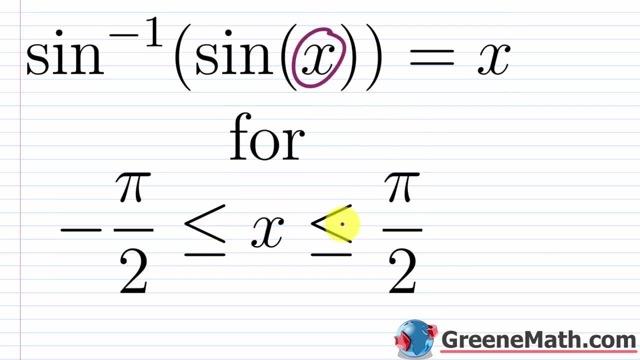 plug in something for x in this interval. right here. you can't just cancel. You'd have to evaluate the sine of x first and then take the inverse sine of that. If you think about it from the other approach, you could say that these guys are only. 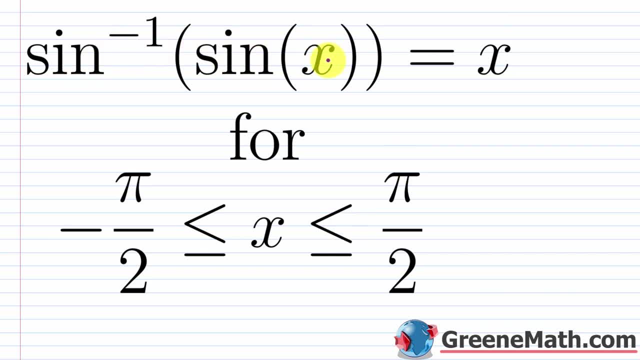 going to undo each other. if you're working with the domain from the restricted sine function, which is where x is greater than or equal to negative pi over two and less than or equal to pi over two, If you're within that domain, well then the inverse sine. 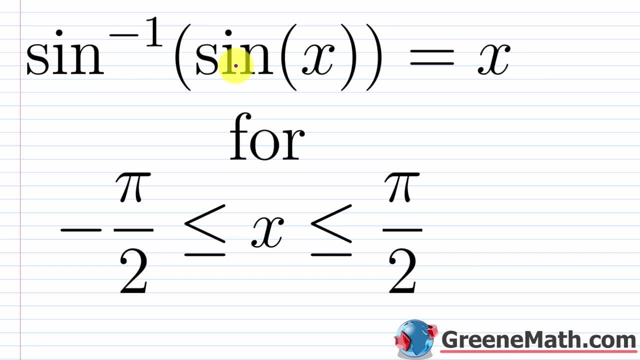 of the sine of x is going to give you x. These guys are going to undo each other. OK, using a similar thought process again when we start with, y equals the cosine of x. it's not a one to one function. 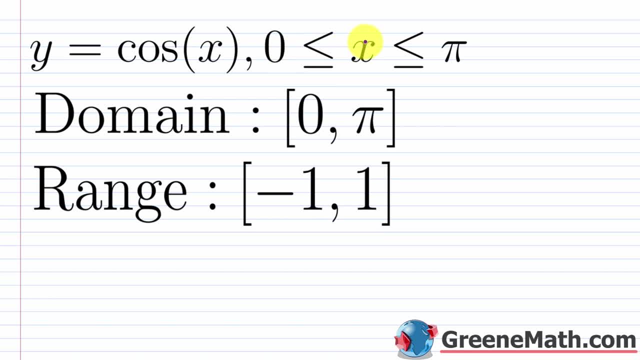 So we restrict the domain to where x is greater than or equal to zero and less than or equal to pi. You're going to have the same range, So from negative one to positive one, both being included. So, again, if you start with that restricted cosine function, 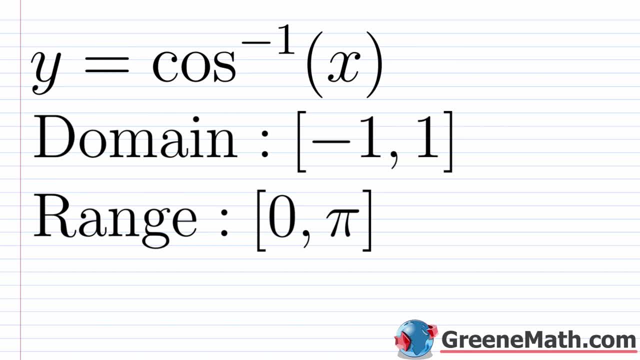 and you swap the x's and the y's, you're going to get your inverse cosine function. So y equals inverse cosine of x, or y equals arc cosine of x, if you want to say it that way, Your domain is from negative one. 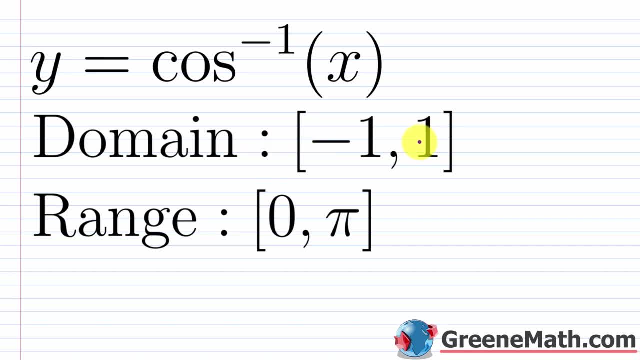 to positive one, both being included, coming from the range of the restricted cosine function. And then the range is from zero to pi, both being included, That's coming from the domain of the restricted cosine function. So here's something like the cosine of the inverse, cosine of x. 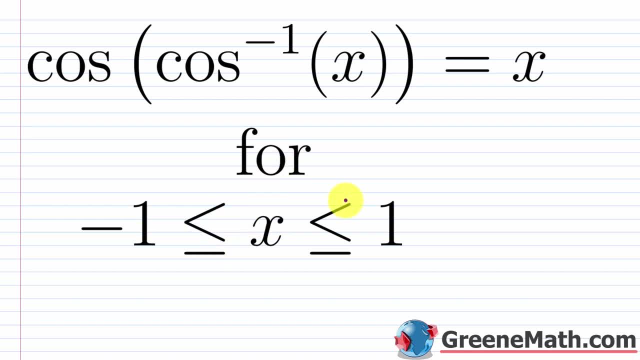 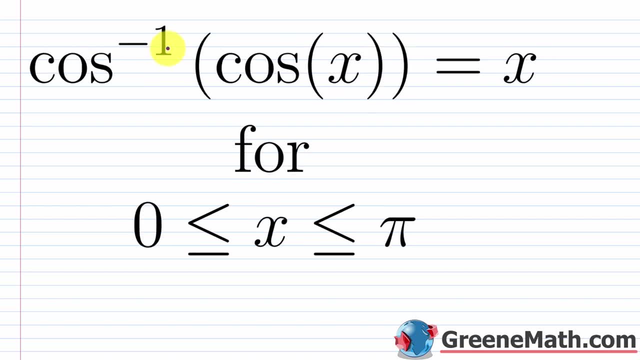 is equal to x, for x being greater than or equal to negative one and less than or equal to positive one. Again, you've got to be within the domain of the inverse cosine function for this to work. And then for this one, the inverse cosine. 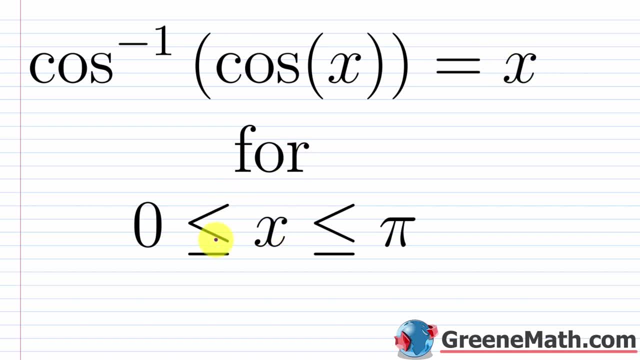 of the cosine of x is going to be equal to x, for x being greater than or equal to zero and less than or equal to pi. So again, you've got to be within the domain of the restricted cosine function for this to work. Again, the other way. 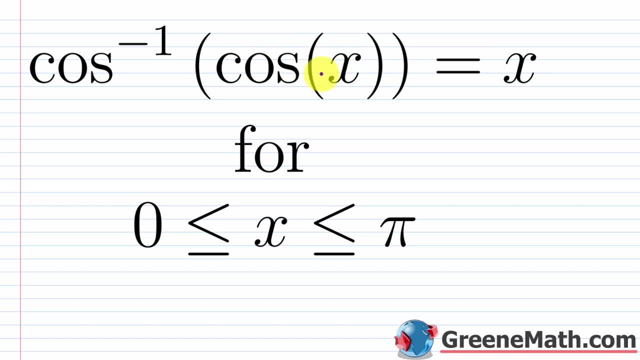 to think about this. you could say that the cosine of x, the domain for that, is all real numbers, So I can plug in whatever I want. But the issue is if it's not in this interval here. I've got to evaluate that first. 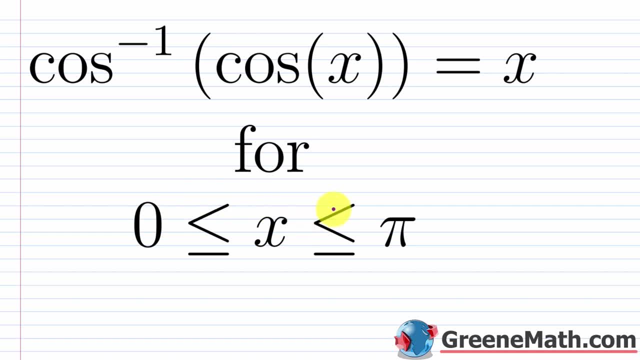 before I take the inverse cosine of it, because the inverse cosine is only going to give me something from zero to pi, with both guys being included. So these guys will undo each other as long as x is in the domain of the restricted cosine function, So again being greater. 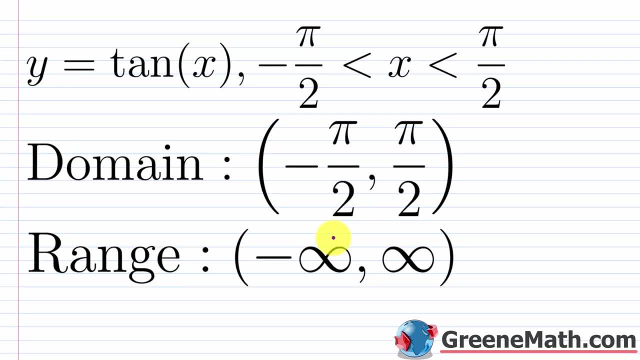 than or equal to zero and less than or equal to pi. And for the last one we look at the tangent of x. So y equals the tangent of x. Again, not a one to one function. You restrict the domain to where x is strictly. 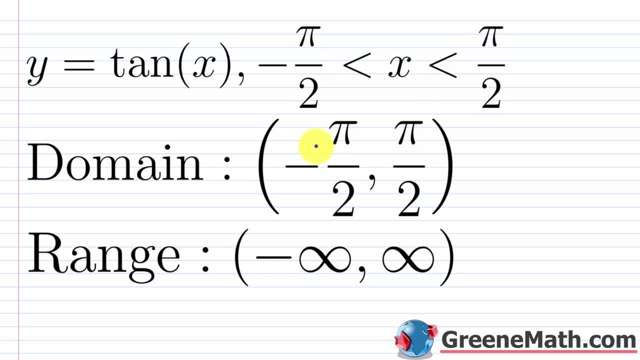 greater than negative pi over two and strictly less than pi over two. So negative pi over two and pi over two are not included. And then when you look at the range, it's going to be all real numbers. So when you swap the x's and the y's, 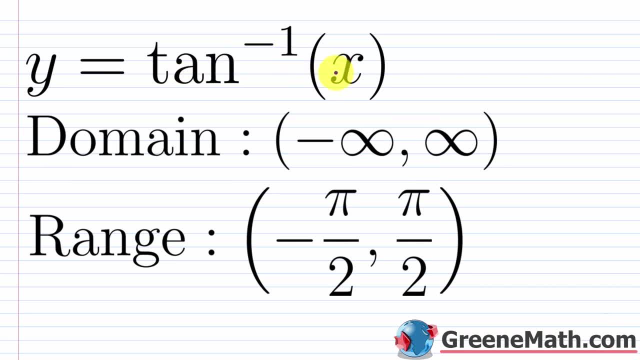 you get your inverse tangent function, So y equals the inverse tangent of x, or y equals the arc tangent of x. So the domain is all real numbers, Again coming from the range of the restricted tangent function, And then the range is going to be: 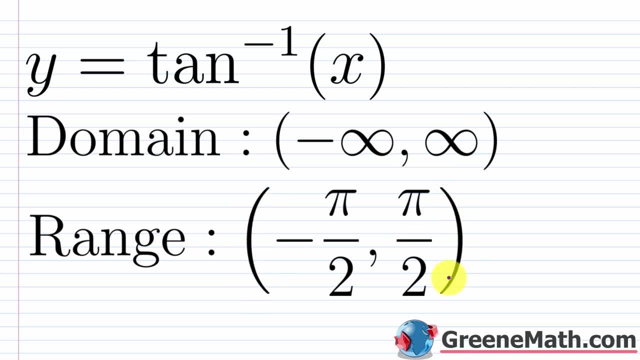 from negative pi over two to pi over two. Again, these guys are excluded here. Remember that the tangent of pi over two or the tangent, the tangent of negative pi over two, those are undefined because the cosine of pi over two is zero. 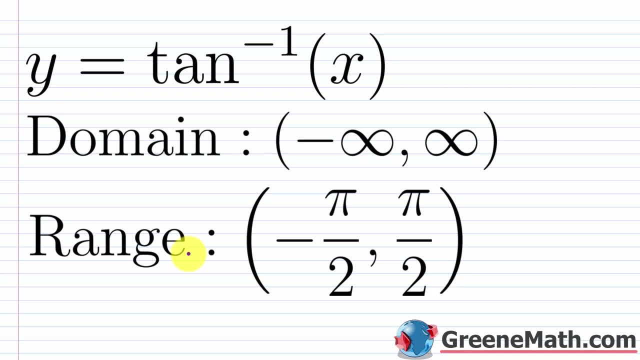 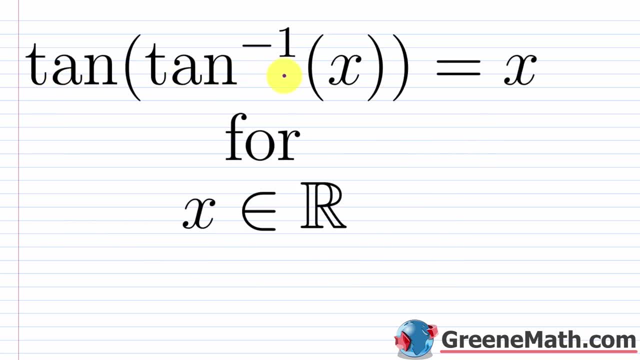 And you'd have division by zero, which is undefined. So when we think about the range here, this is coming from the domain of the restricted tangent function. All right, So this first one's really easy to understand. So the tangent of the inverse tangent of x. 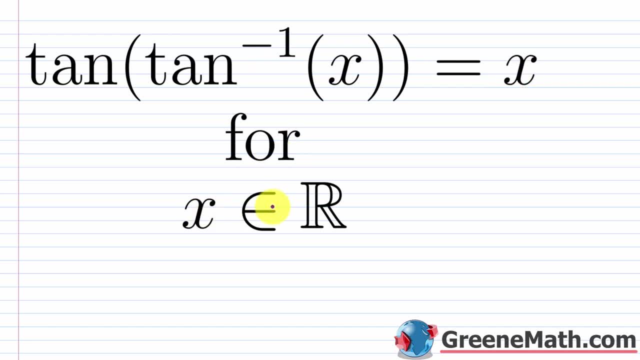 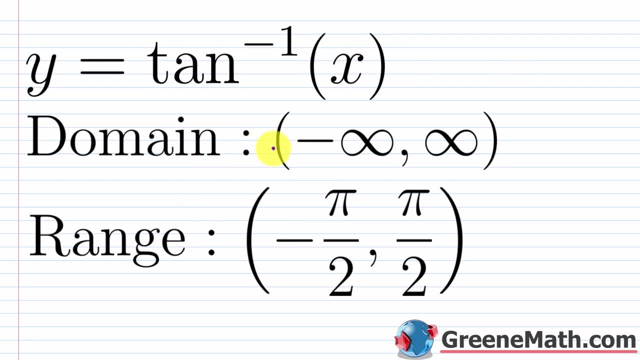 is equal to x. For any x, that is a real number. So that's what this means. This means x is an element of the set of real numbers And basically, if you think about the domain of the inverse tangent function, again it's all real numbers. 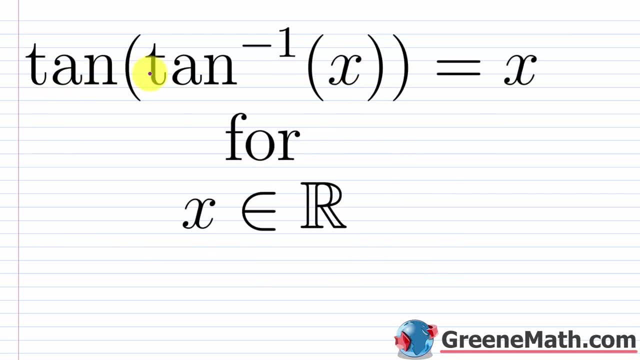 So that's why we can plug in whatever we want here And these guys, these guys will undo each other. When we think about this one again, this is the one that's more tricky to understand. So the inverse tangent of the tangent of x. 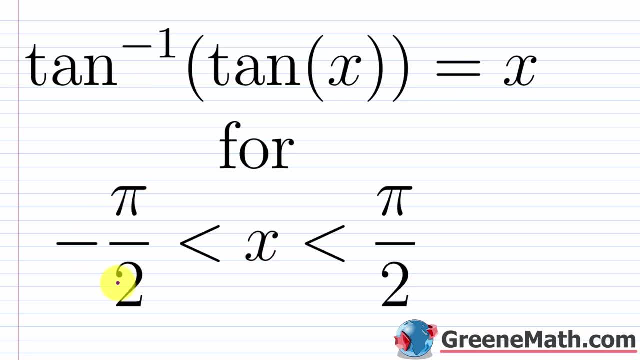 this is equal to x, for x being greater than negative, pi over two and less than pi over two, So this x is going to be in the domain of the restricted tangent function. if you want these guys to undo each other, All right, Let's take a look. 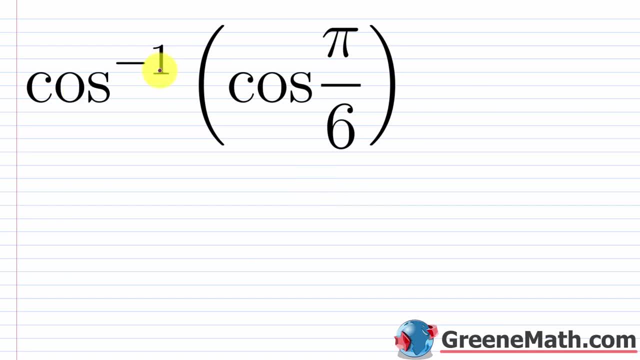 at a few sample problems. So suppose you're given the inverse cosine of the cosine of pi over six. The first question you would ask is: is this angle pi over six, in the domain of the restricted cosine function? If it is, these guys are going. 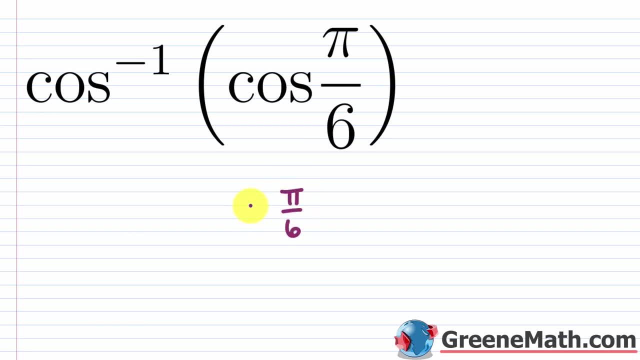 to undo each other. So, in other words, is pi over six greater than or equal to zero? Well, yeah, that part's true. And less than or equal to pi? Well, yeah, that's true as well. So I can go ahead and say: 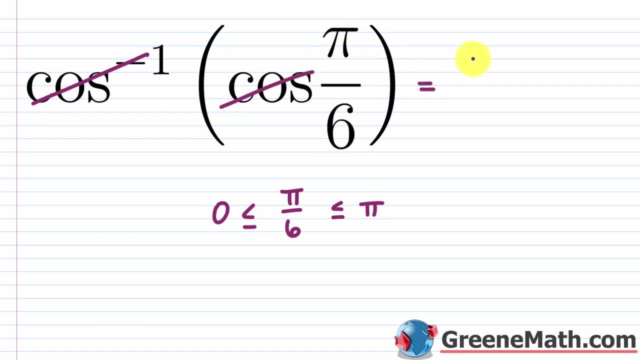 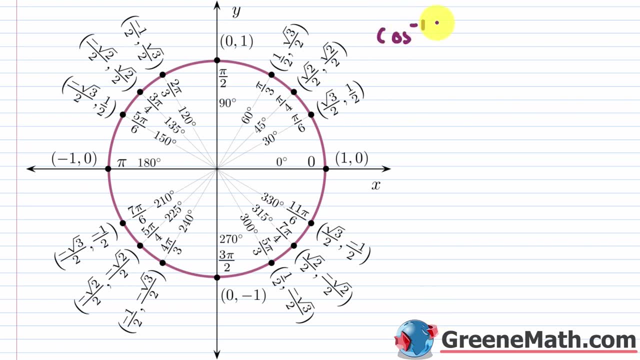 that this would cancel away with this and I'm just left with that pi over six. So that's going to be my answer. If you wanted to look at this on the unit circle again, you would start. let's say we had the inverse cosine. 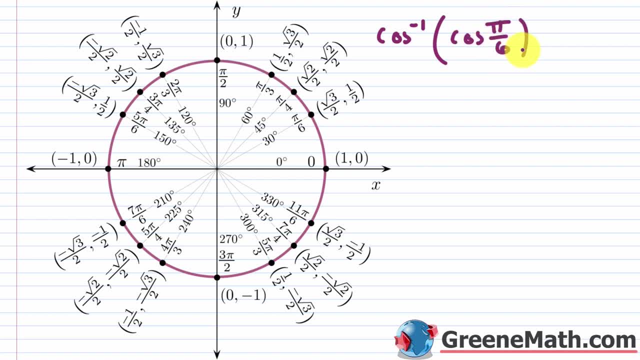 of the cosine of pi over six. And we're going to do this the long way. So we're going to start on the inside And basically we would say: what is the cosine of pi over six? So I come to pi over six. 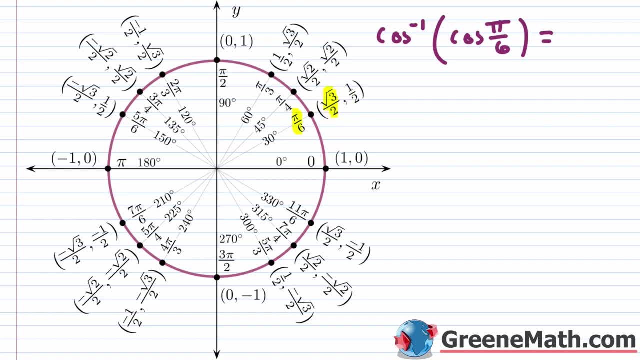 That's right here. The x coordinate is my cosine value, So that's square root of three over two. So now we want the inverse cosine of the square root of three over two. When I think about the inverse cosine function again, I'm going to work. 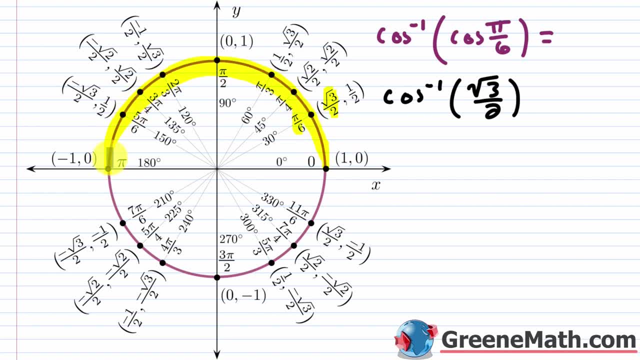 from zero to pi, where zero and pi are both included. So I'm just going to ask the question: what angle has a cosine value of square root of three over two in this interval from zero to pi, where zero and pi are both included? Well, we already know. 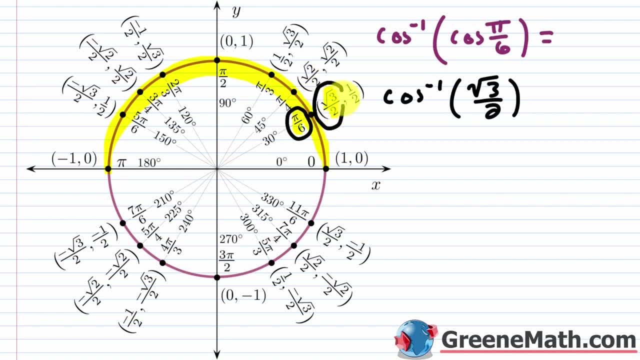 that that's going to be pi over six. Here's your cosine value of square root of three over two. So you're just reversing what you just did. You found the cosine of pi over six and that was square root of three over two. 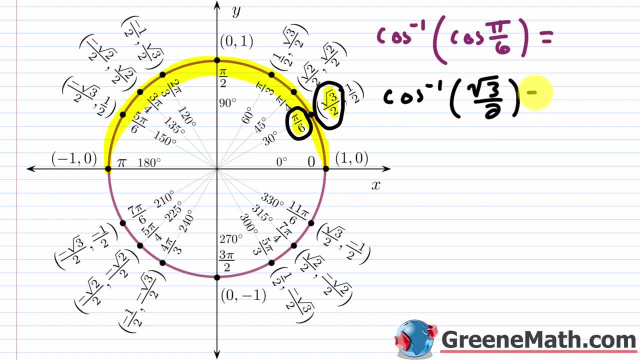 Well now the inverse cosine of square root of three over two is going to get you back to pi over six. So this, right here, is your answer. And again, if you see something like the inverse cosine of the cosine of pi over six, 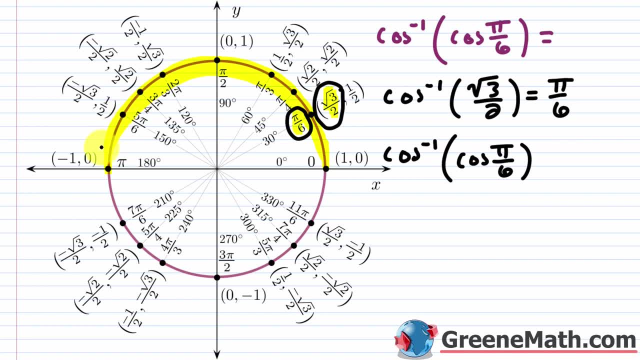 because this pi over six is in the domain of the restricted cosine function, or you can also say the range of the inverse cosine function. you can go ahead and just shortcut this process and say this is going to cancel with this. So they'll undo each other. 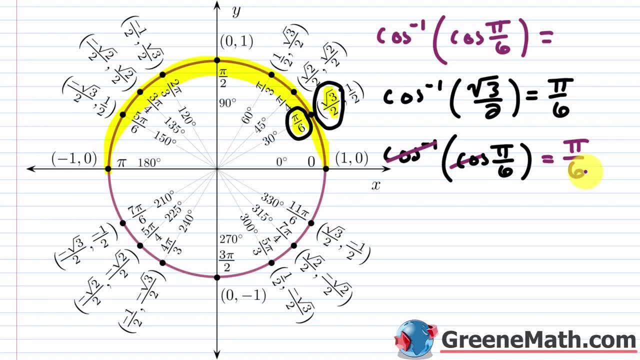 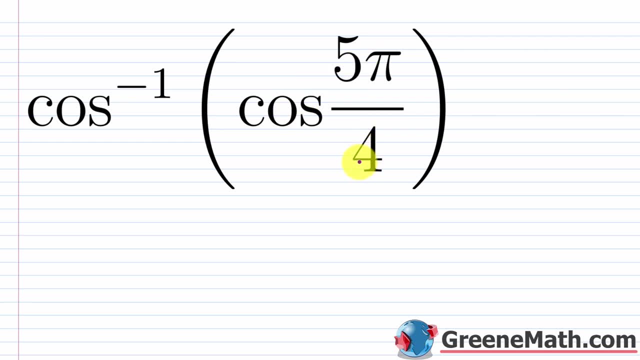 and you're going to be left with this pi over six as your answer. Okay, let's look at another example. So here we have the inverse cosine of the cosine of five pi over four. This is the one where a lot of people would make a mistake. 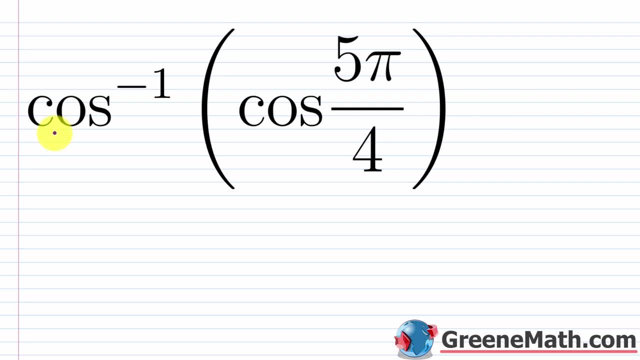 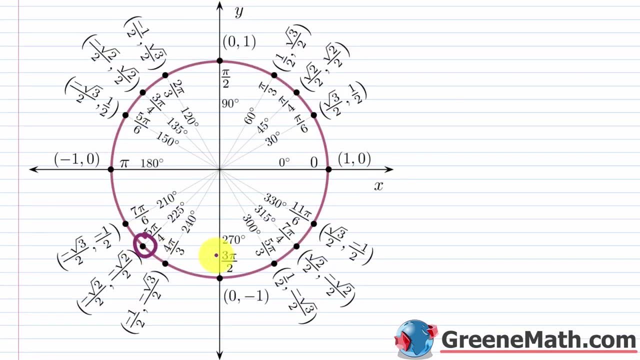 So if you give the answer as five pi over four, that is incorrect. In other words, you can't just cancel here because this five pi over four if you go to the unit circle, that's going to be right here. So that is not going to be correct. 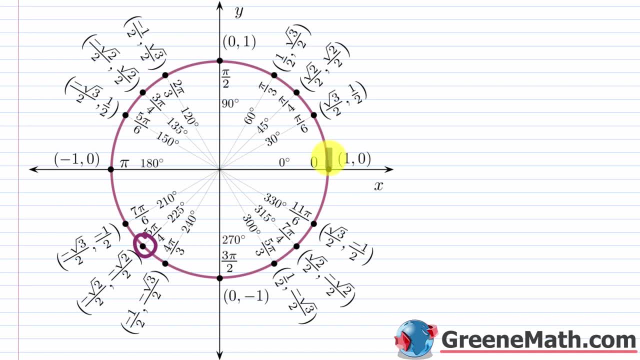 It's not within the domain of the restricted cosine function or the range of the inverse cosine function. Again, you're thinking about this from zero to pi, where both zero and pi are included. So what you have to do for this particular problem, 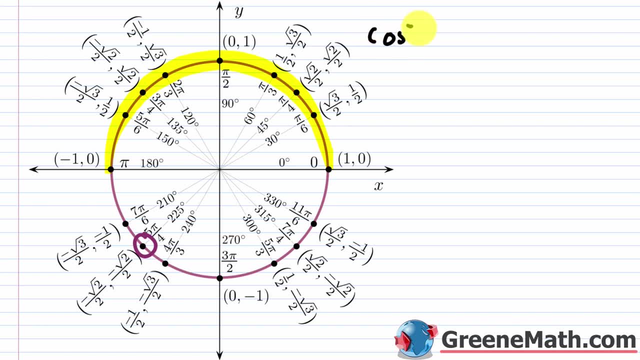 you have to go about it the long way. So you have to say: this is the inverse cosine of the cosine of five pi over four. Okay, so what is the cosine of five pi over four? Well, if I come over here, that's going to be. 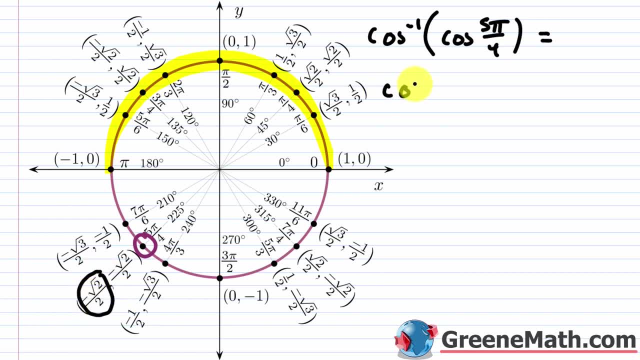 the negative of the square root of two over two. Okay, so now I have the inverse cosine of the negative of the square root of two over two, Okay, so what is the inverse cosine of the negative of the square root of two over two? 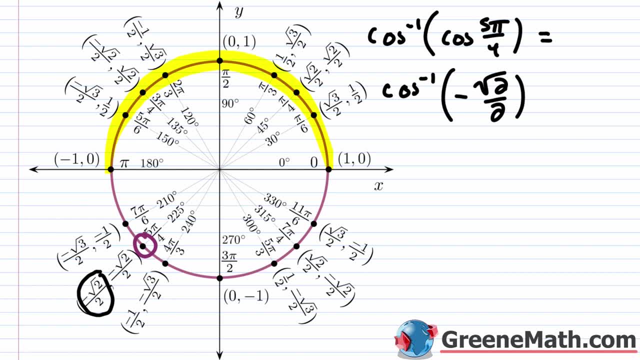 So if this guy is negative, I want to be in quadrant two where cosine is negative And I'm looking for where I have a cosine value of negative square root of two over two. So that's going to be right here And that's going to be at three pi over four. 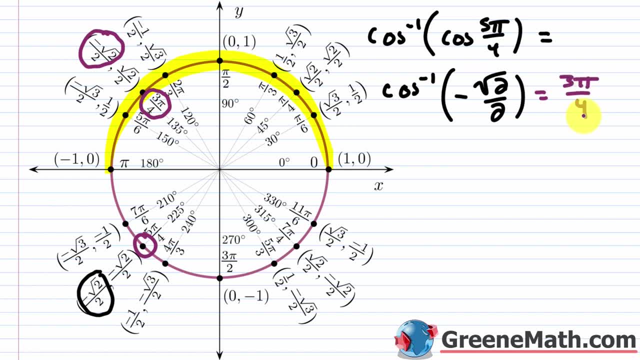 So this would be equal to three pi over four. Now if you had gotten the inverse cosine of the cosine of three pi over four again, because this three pi over four is in the domain of the restricted cosine function, or you could say the range, 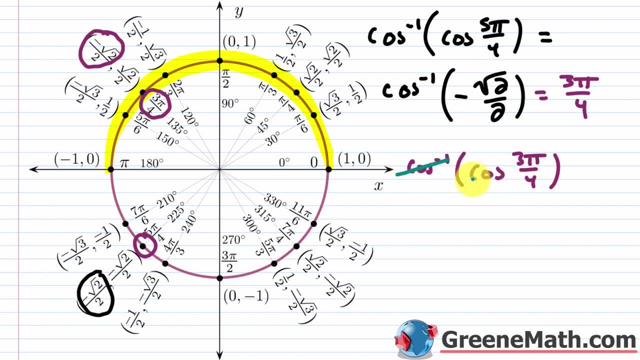 of the inverse cosine function in this particular situation. you can cancel this with this. Those will undo each other And then basically you're left with that angle of three pi over four. When you get a situation like this because this is not within the domain, 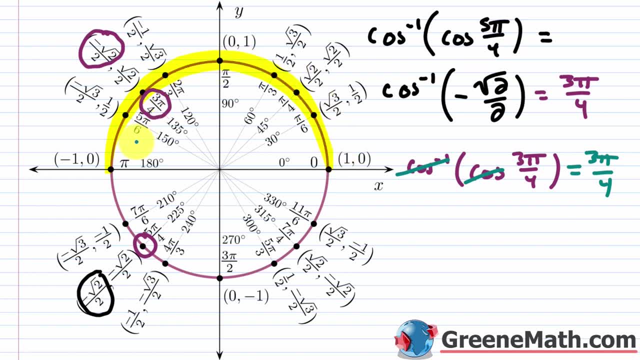 of the restricted cosine function or the range of the inverse cosine function. you have to do more work. You have to first evaluate the cosine of five pi over four, which is negative square root of two over two. Then you take the inverse cosine of negative square root of two over two. 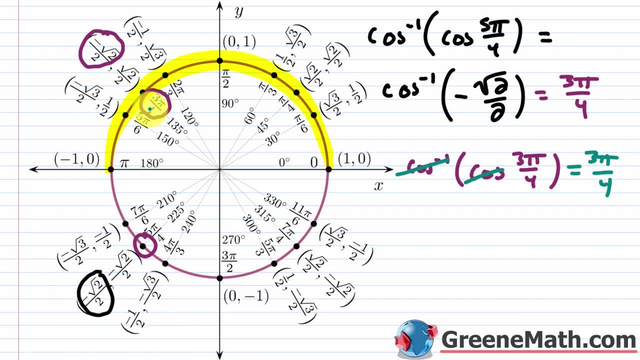 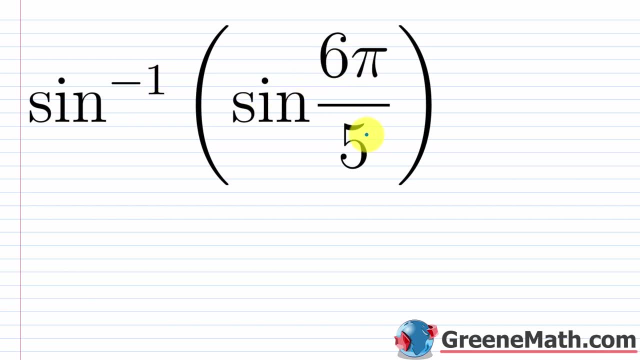 And that's going to give you this angle in quadrant two, which is three pi over four. All right, let's take a look at one more of these. So here we have the inverse sine of the sine of six pi over five. Now, when we get this problem, 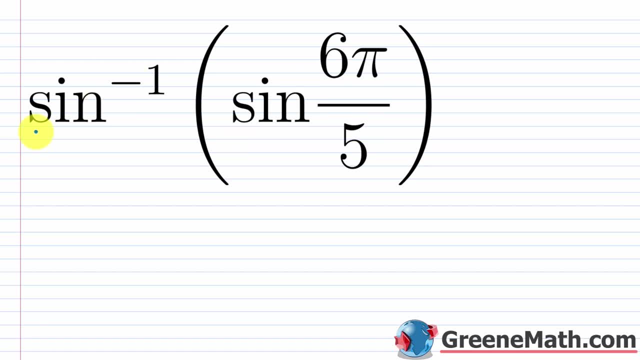 again. I'm always asking: is this guy going to undo this guy? In other words, are these guys going to cancel away and just give me six pi over five as my answer? And here you're going to say no, because for this to work that way, 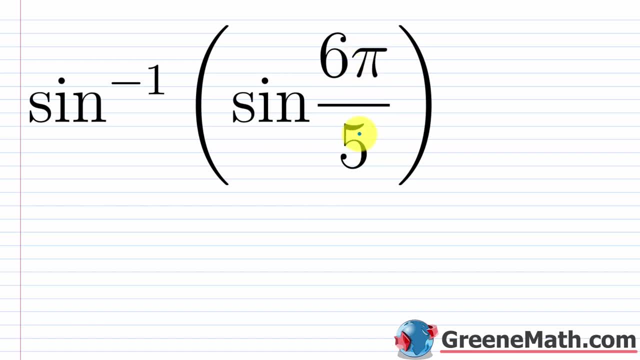 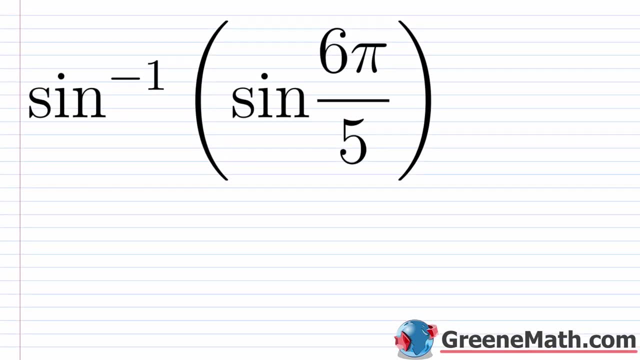 you have to have this six pi over five being in the domain of the restricted sine function or the range of the inverse sine function, And it's not. If you think about, let's say, the range of the inverse sine function, again you're working. 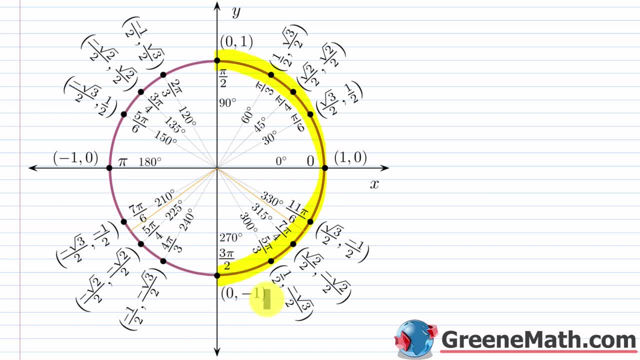 from negative pi over two to pi over two. So you've got to be there. When you think about six pi over five, that's not directly on the unit circle. I've sketched it in, So let me put six pi over five. 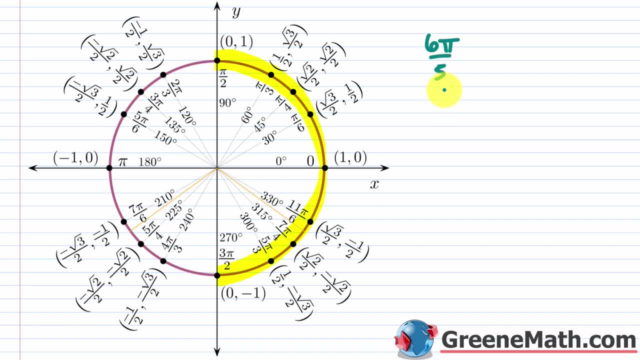 And you might be scratching your head, saying, well, where's that angle at? And you can do some analysis and think about, okay, well, it's going to end up being in quadrant three. So I'm just going to write this one out. 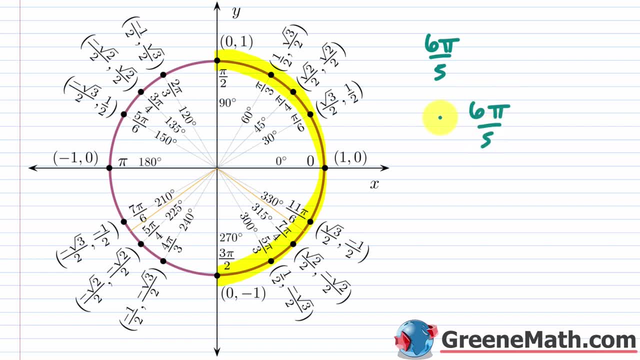 And I'll give you an easier way to do that by converting it. So I'm going to write this one out. So this would be greater than pi and less than three. pi over two. So that tells me I have an angle in quadrant three. 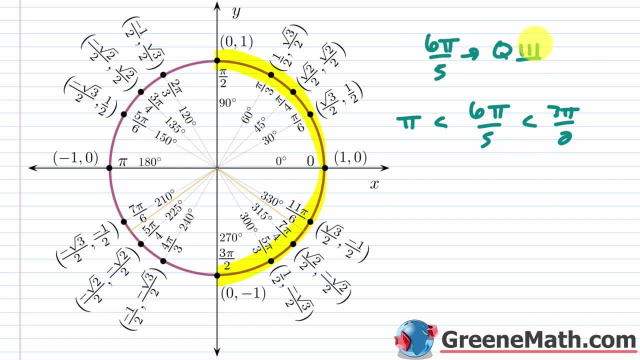 So let me just put that this is in quadrant three. Now, an easier way to do that. if you're struggling with that, you can always convert it over into degrees. Way easier to do. So I'm just going to say it's six pi over five times. 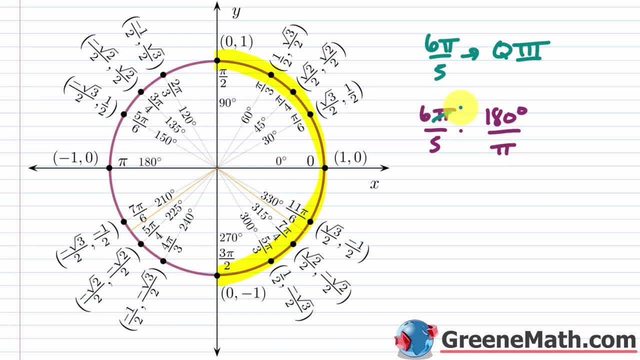 I'm going to go 180 degrees over pi, And so basically the pi's are going to cancel. And so 180 divided by five is 36.. And so you'd have six times 36. That's 216.. And now this is in terms of degrees. 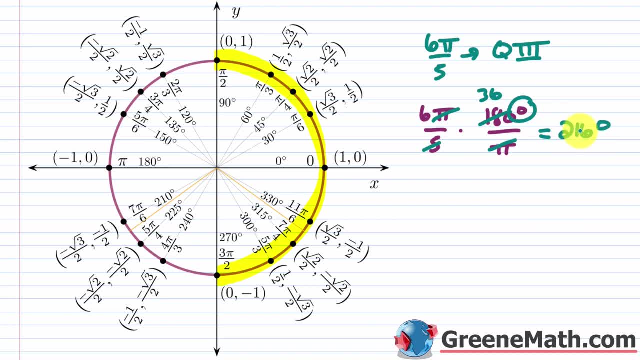 So this is 216 degrees, So I think a lot of people will find this easier to work with And also immediately. you know that this is going to be in quadrant three, Whereas with six pi over five. you really have to think about it. 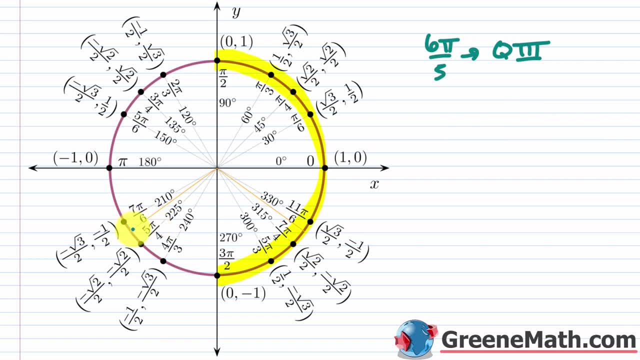 because it's in terms of radians. I've already sketched this in to help us out. So this guy in orange, which I'm not sure if it comes through so well. So I'm going to try to do a rough trace over what I did. 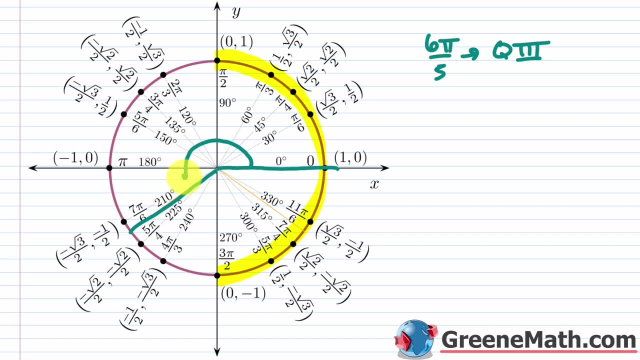 So this would be your angle right here. So this is what I'm looking at. So that's my six pi over five. Now I know that the sine of six pi over five is going to be negative because it's in quadrant three. I also know that the reference angle 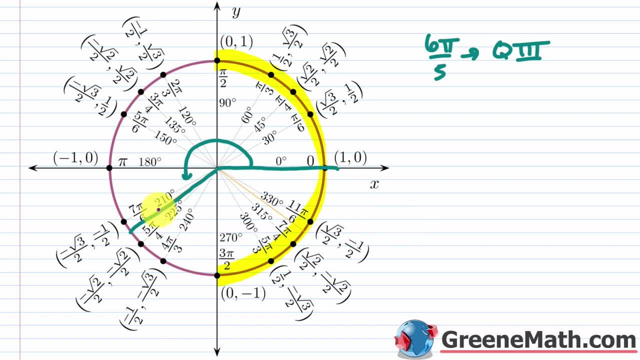 is going to be pi over five, And the way I figure that out is: if I'm in quadrant three, I take my angle, which is six, pi over five, and I subtract away pi, So I'll do that as five, pi over five. 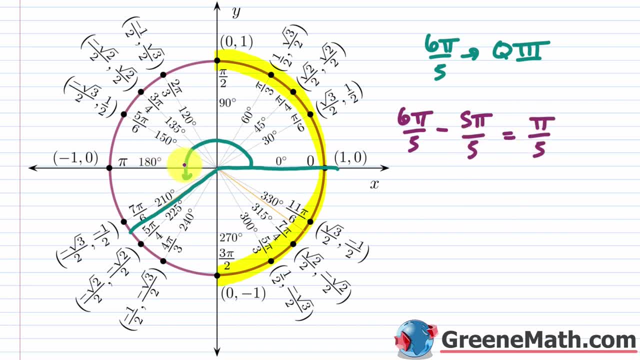 And that gives me pi over five. So this guy right here, this reference angle, so this piece right here, that's going to be pi over five. Now I know that sine is negative again in quadrants three and four. So all I have to do 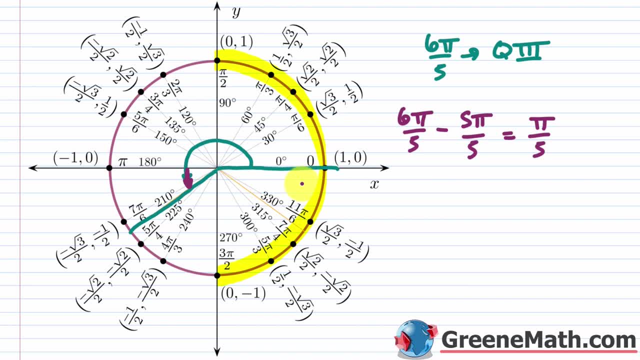 is come over into quadrant four and find an angle with a reference angle of pi over five. But again, I don't want to do this. I don't want this angle right here, because I want to rotate clockwise in quadrant four when I have a negative argument. 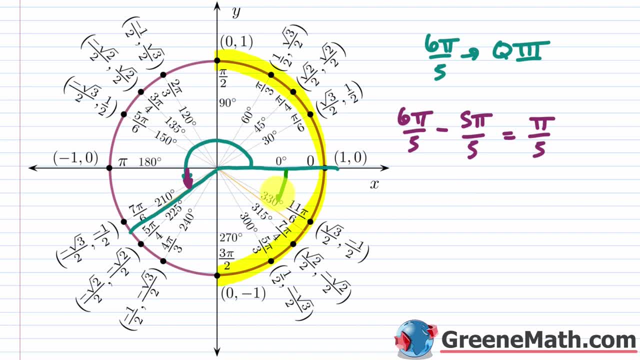 for my inverse sine function. So I want this guy right here, right here. So I'm going to draw over this, maybe use a different color. So this guy right here, that is going to be negative pi over five. So I've got my pi over five. 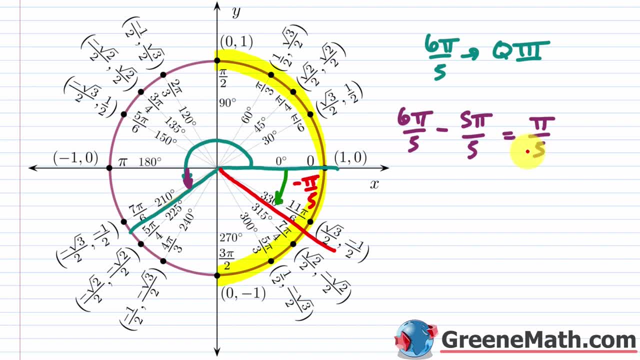 reference angle. So now I want to convert my problem over to where I use something that's going to be in the range of the inverse sine function. So let me get rid of all of this. I think we're ready to go, And all we have to do now is say that. 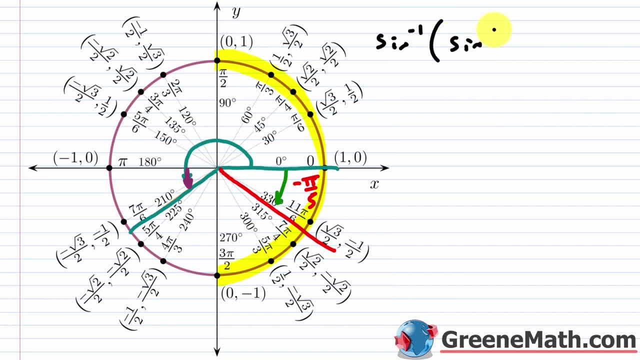 the inverse sine of the sine of six pi over five would be equal to the inverse sine of. again, I'm going to convert this over into an angle that's in the range of the inverse sine function And so I'm going to say it's the sine. 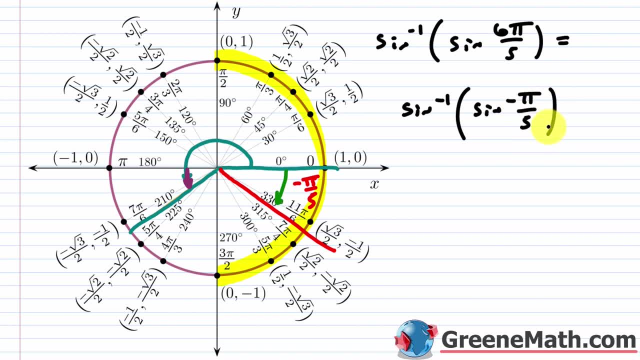 of six pi over five, Of negative pi over five, Because, again, the sine of six pi over five and the sine of negative pi over five, those are both going to be the same value. They're both in quadrants where sine is negative. 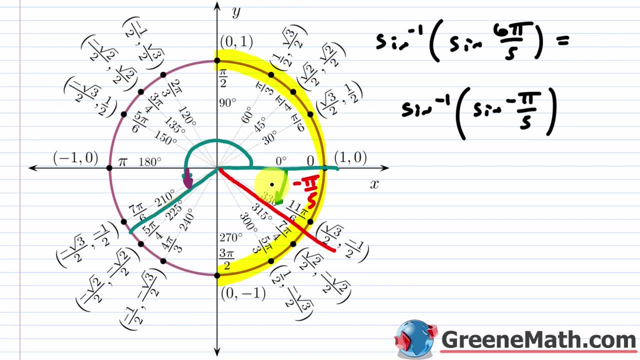 So they're negative in quadrants three and four And the reference angle is pi over five in each case. So all I have to do now is give my answer, as these guys are going to cancel and I'm left with that angle, which is negative: pi over five. 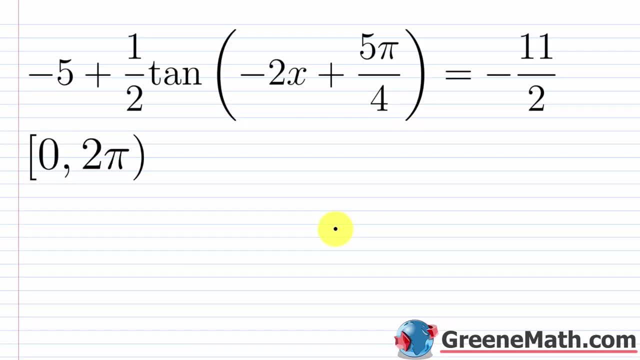 All right, let's take a look at a few examples where we're going to solve some trigonometric equations using inverse trigonometric functions, The cancellation properties that we talked about earlier. So suppose you had something like negative five plus one half tangent of negative two X. 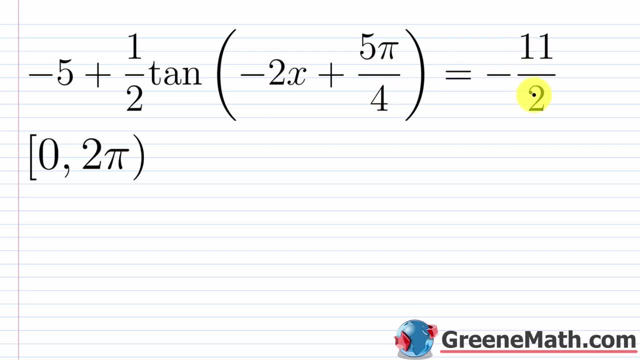 plus five pi over four And this equals negative 11 halves. Now we want to solve this over the interval from zero to two pi, where zero is included and two pi is excluded. Now, earlier in the section we talked about how we could solve: 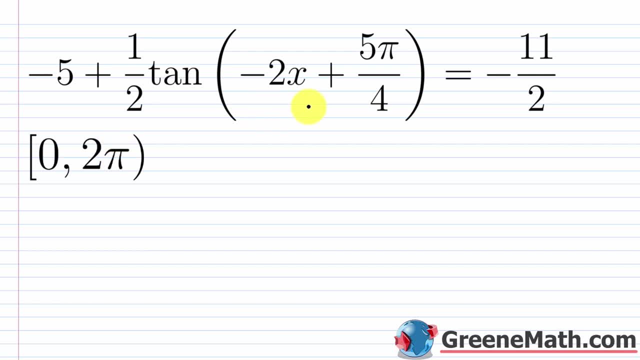 equations of this form, But here we're going to use a different approach, So let me copy the problem. So negative five plus one half, And then we have our tangent of this- is negative two X plus five, pi over four, And this equals negative 11 halves. 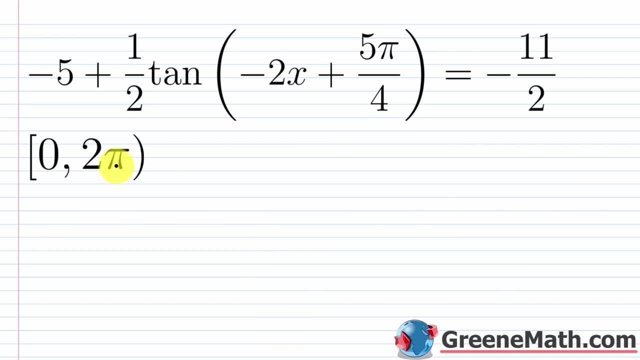 So let me go ahead and grab this real quick. Just remember the interval that we're solving over. I'm going to come here to a fresh sheet, So we have a little bit of room to work. So the idea here is still the same. 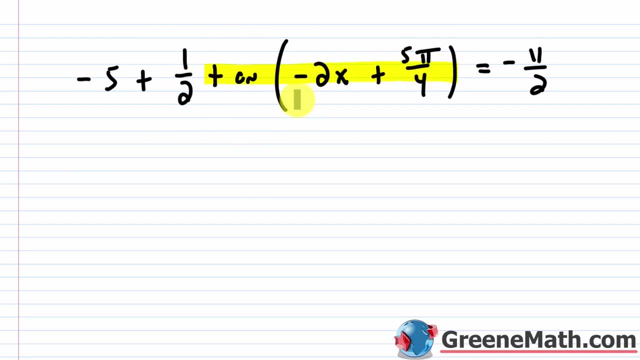 You want to isolate the tangent of something. In this case it's negative. two X plus five, pi over four. So we want to isolate that on one side. You want a number on the other, So what I'm going to do is add five. 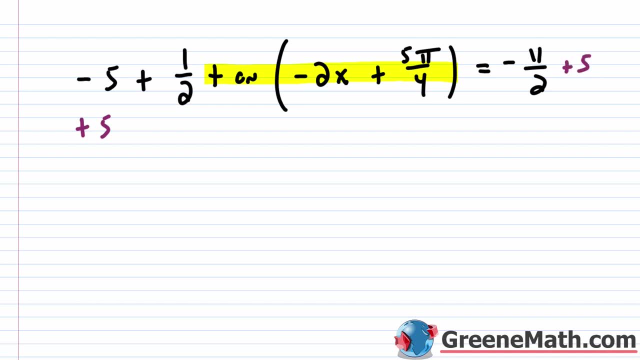 to both sides of the equation. So over here this is going to cancel away And I'm going to have one half tangent of negative two X plus five pi over four And this would be equal to. over here I have a negative 11 halves and then plus for five. 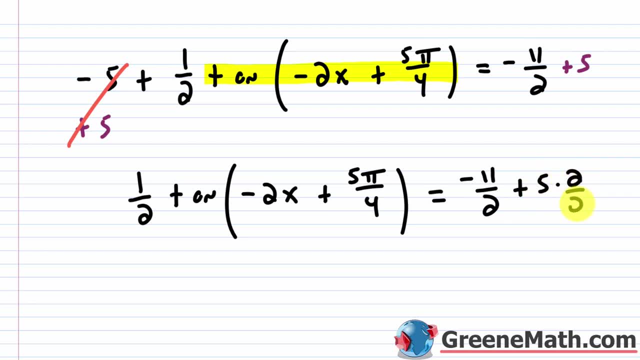 Let's write that with a common denominator. So let's multiply by two over two, So this would be 10 halves, And then now I can add negative 11 plus 10. That's negative one. Put that over the common denominator of two. 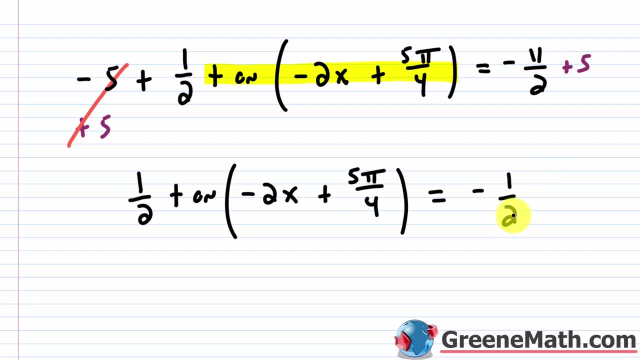 So this would get me, So this would give me negative one half. Now again, if my goal is to isolate this guy right here, I have to think about the fact that I have that one half. that's multiplying that. So to get rid of that, I'm going to multiply both sides of the equation by two. 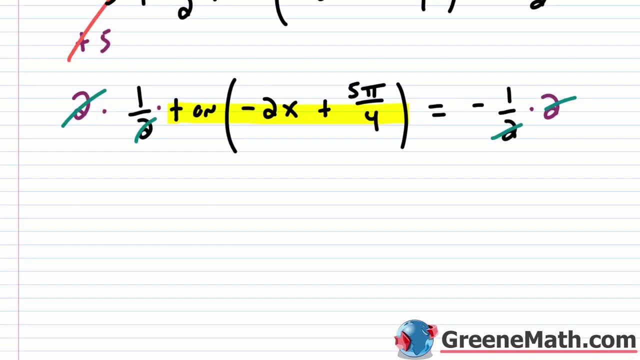 And so this is going to cancel, and this is going to cancel. And so at this point, what I have is the tangent of this: negative two X plus five, pi over four, And this equals over. here I just have my negative one. So here's where we're going to do this. 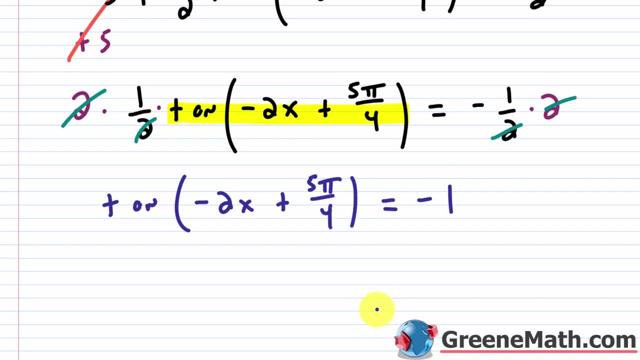 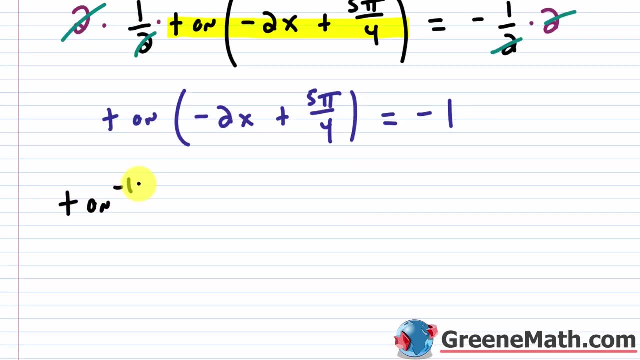 We're going to use our inverse tangent function and the cancellation property that we talked about earlier, So I'm going to take the inverse tangent of each side. So let's start over here. I'm going to say that I have the inverse tangent of this guy right here. 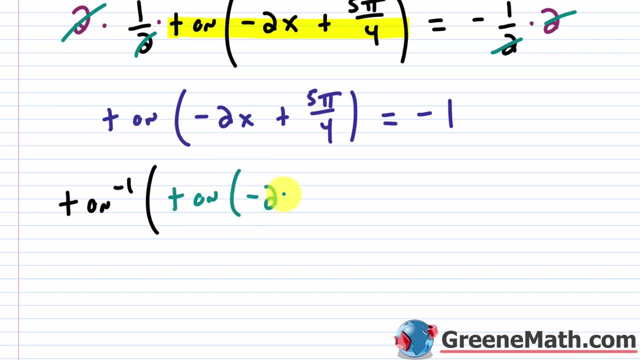 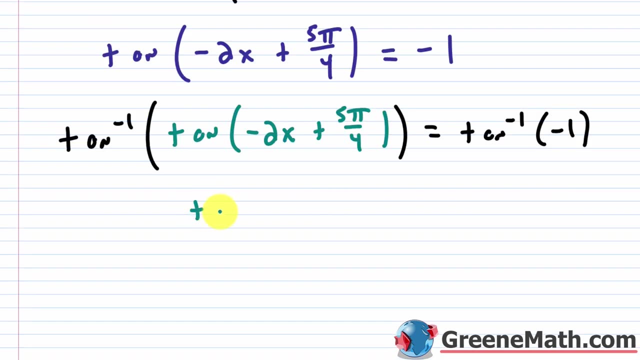 So this would be the tangent of negative two X plus five, pi over four. And then this guy over here on the right, you're going to do the same thing. So I'm going to take the inverse tangent of this negative one. Now, again, we have our property where we said: 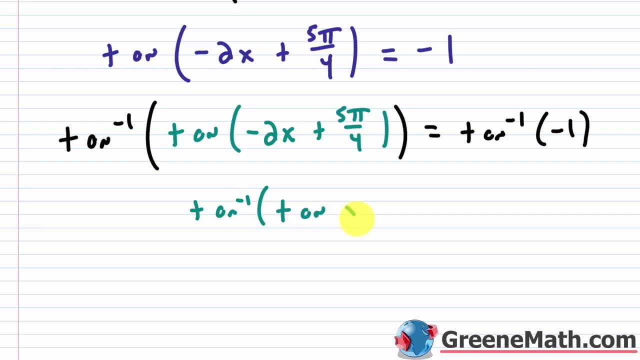 that the inverse tangent of the tangent of X, in this case X, is just this guy right here. So this is what's on the inside. We would say that this is equal to X as long as X is greater than negative pi over two and less than pi over two. 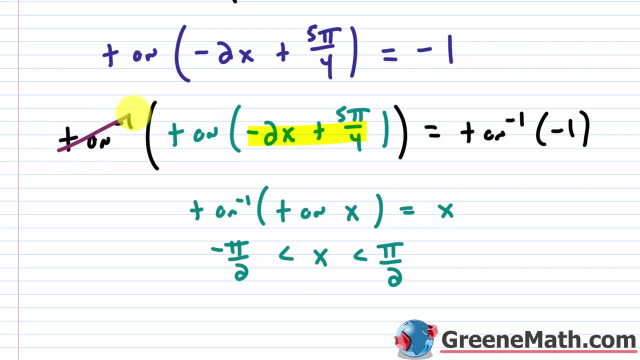 So we're going to use this property here And basically we're going to say that this guy and this guy are going to undo each other or cancel each other, However you want to think about that, And so I'm just going to be left with this part, right here. 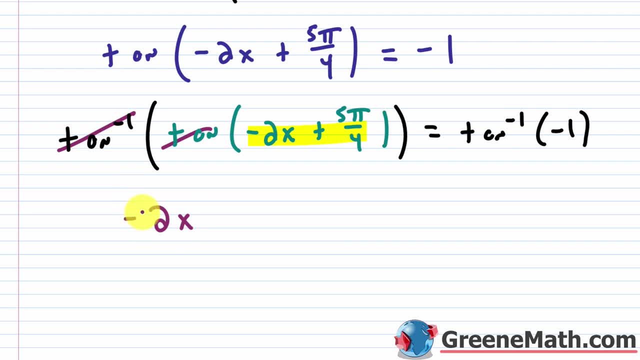 So I'm going to say this is negative two X- Let me move this down a little bit More- and then plus five pi over four, And this equals the inverse tangent of negative one. Now, most of you know that's negative pi over four. 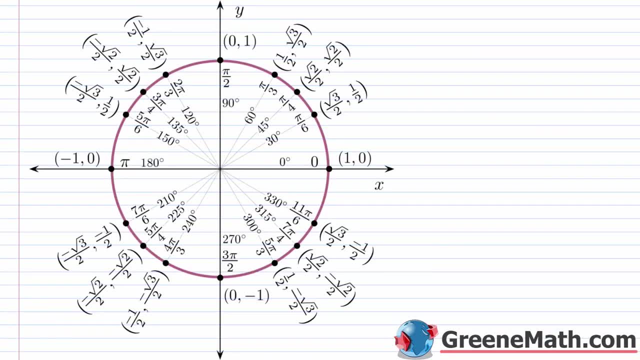 But just in case you don't again, you can always go to the unit circle and think about these things. So for the inverse tangent function, again you're working from negative pi over two to pi over two, with those values being excluded. 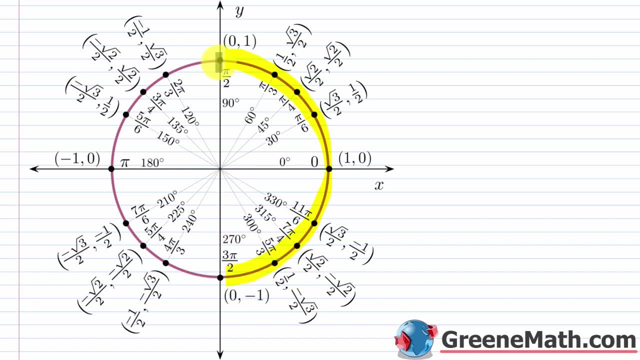 So I'm going to make sure that I stop a little bit short there, So those guys are not included. Again, the negative pi over two and the pi over two. And you're just asking the question: where, in this interval here, Am I going to have a tangent value? that's going to be negative one. 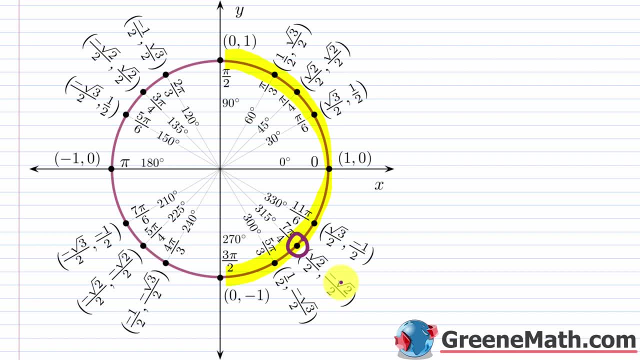 Well, a lot of you can see that at seven pi over four you have a sine value- that's negative square root of two over two, and a cosine value that's square root of two over two. So if you have the tangent of seven pi over four, you're dividing opposites. 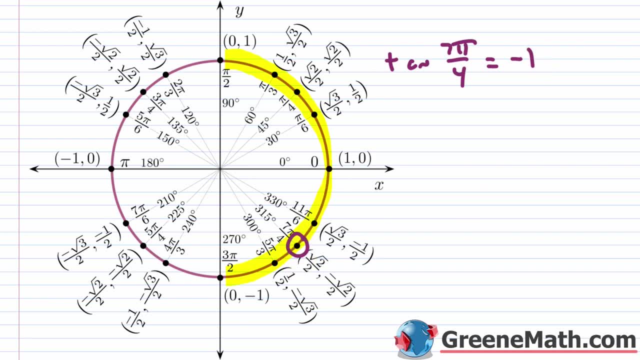 So that's equal to negative one. Now we can't put seven pi over four because again we have to rotate clockwise here, So you've got to go like this. So this would be negative pi over four And of course that's coterminal with seven pi over four. 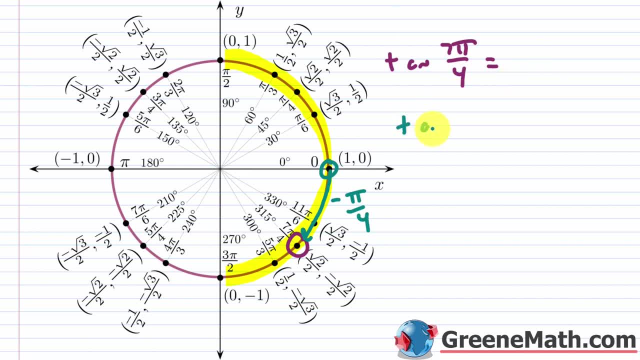 So the tangent of seven pi Four is equal to the tangent of negative pi over four, And that equals negative one. So if I took the inverse tangent, so the inverse tangent of negative one, that's going to give me this negative pi over four. 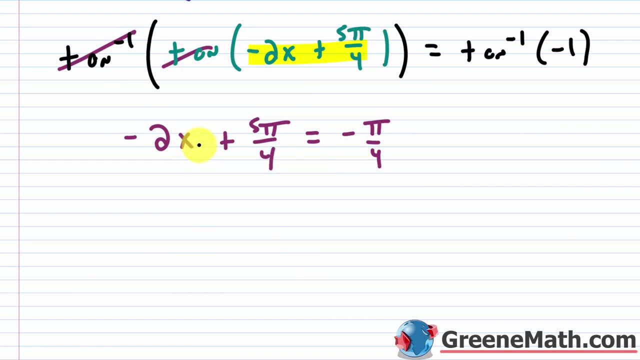 OK. so coming back to this point, what we want to do is solve for X. So now I have this guy that I want to isolate. So let's subtract five pi over four away from each side of the equation, So of course this is going to cancel. 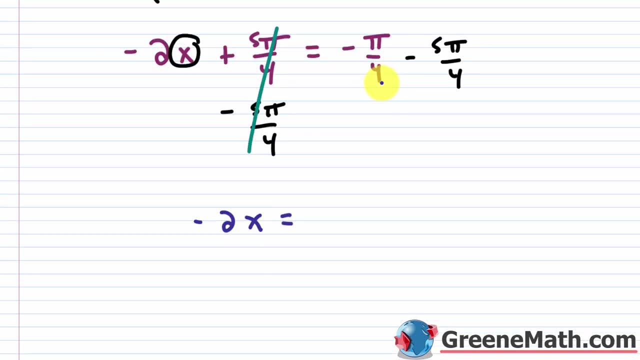 And now I'm going to have negative two X is equal to- Let's write this as Negative pi minus five pi over the common denominator of four. So this right here, negative pi minus five pi, is negative six pi. So this is going to be negative six pi over four. 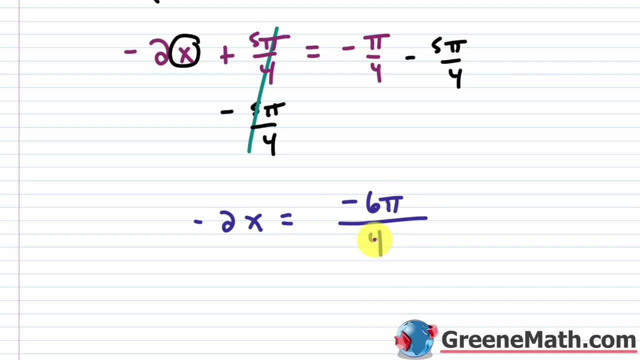 Now to simplify this: if you think about six and four, there's a common factor of two. So six divided by two is three, and four divided by two is two. So let's go ahead and write this as negative. three pi over two. 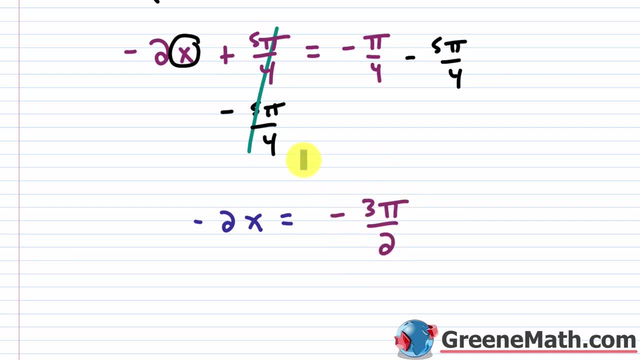 So this is negative three pi over two. Now, as a last step, again, I want to isolate X. So what I want to do is think about the fact that negative two is It's multiplying X, so you can divide both sides by negative two. 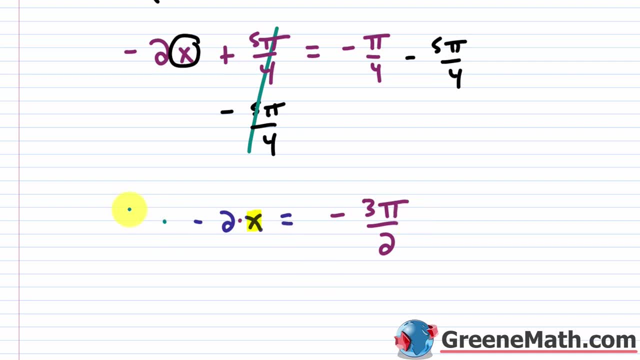 Or, since you have a fraction here, it's probably going to be a little bit easier if you multiply both sides by negative one half. So multiply both sides by negative one half. So of course you could write this as negative two over one. 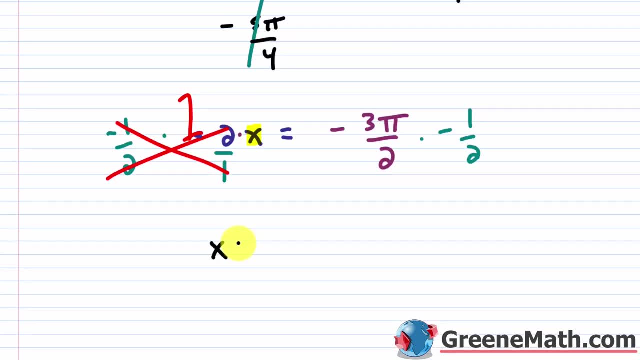 And this right here would cancel and become a one, And so you would have: X is equal to negative times, negative is positive, And then basically you would have three pi over four. So that is only one solution, And that's part of the issue with this technique here. 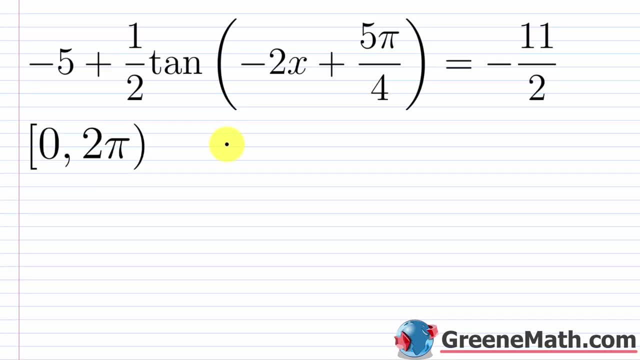 So you have: X equals three pi over four. So let's go back up to the top and let me write that X is equal to three pi over four. So I know that this guy right here is in quadrant two. You're going to find that you actually have a solution in quadrant one, two. 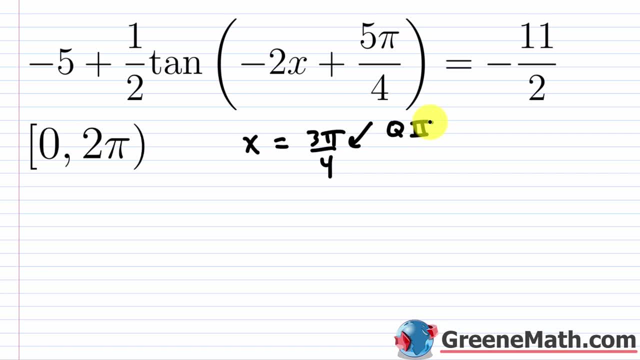 three and four with this problem And the way I know that is, I would look at the period of this guy, So I know how often these solutions are going to repeat Again. the standard period for tangent is going to be pi. When you look at, Y is equal to the tangent of X. 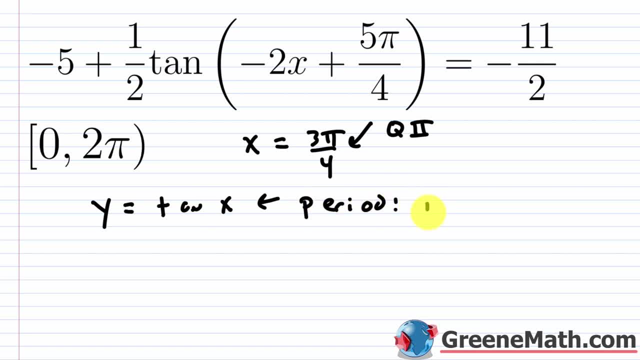 Well, the period for that guy, the period for that guy is going to be pi, But if you have Y is equal to something like the tangent of BX. well then, the period, So the period is now going to be pi over B. 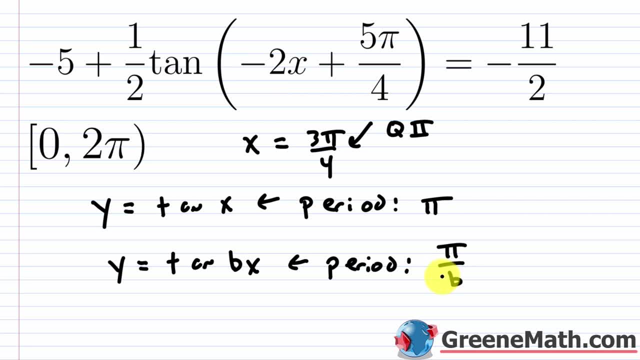 But that's when B is positive. In this case you're going to have a negative here, So you can adjust the formula and say pi over the absolute value of B. So for this case you have this negative two, that's multiplying X. 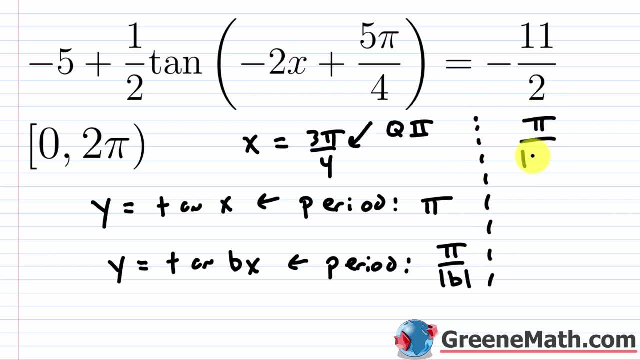 So the period for this guy would be pi over the absolute value of negative two, which would be pi over two. So that's going to be the period. Let me get rid of this. So let me put this like this, and let me put that the period period is pi over two. 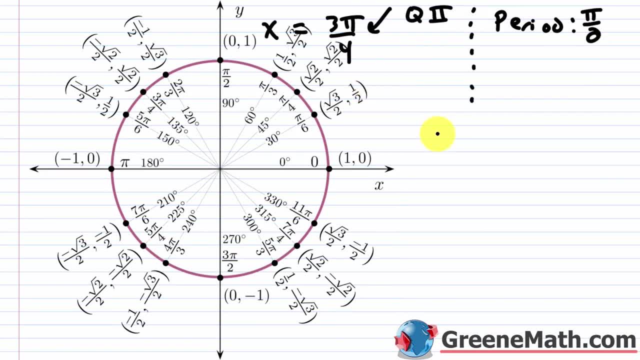 And actually let me grab this real quick. It's going to come down here to the unit circle and rewrite things. So X is equal to three, pi over four. Again, this is in quadrant two and I'm going to put that the period. 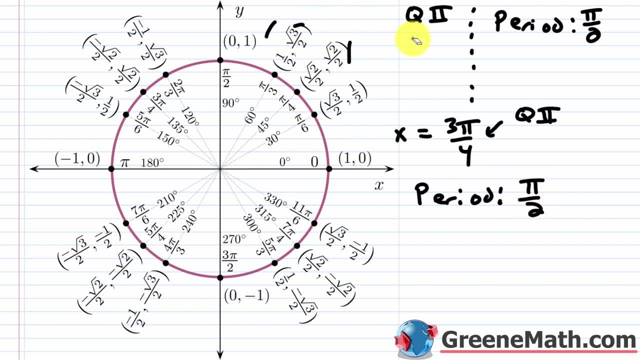 So the period is pi over two. I think you can do it on the unit circle the first time, just so you can get a visualization of what's going on. So I know that solutions repeat every pi over two. So here I'm going to be at three, pi over four. 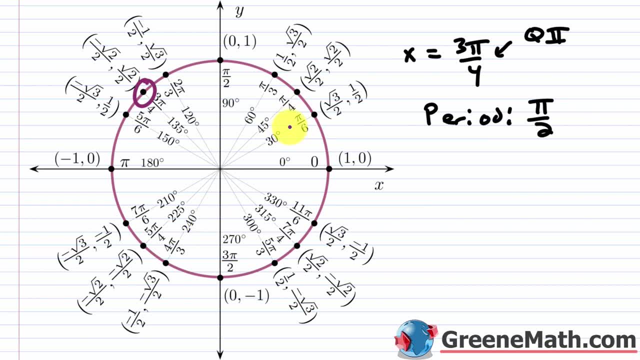 What I want to do is actually subtract away pi over two and find my solution in quadrant one. A lot of you know that's going to be pi over four. Well, let's go and do the work here. So we have three pi over four minus pi over two. 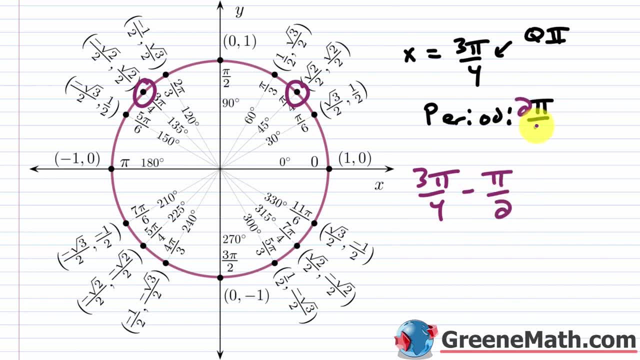 Let's go ahead and write this as two pi over four, So we can have a common denominator. So minus two pi over four, And so this would give me again pi over four. So that's a solution in quadrant one. Now, if I want the solution in quadrant three, 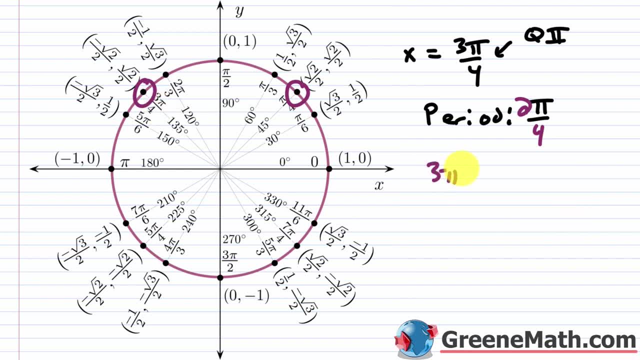 then what I would do is actually take my three pi over four, So three pi over four, And I'm going to add two pi over four And that's going to give me five pi over four. That's going to be right here. 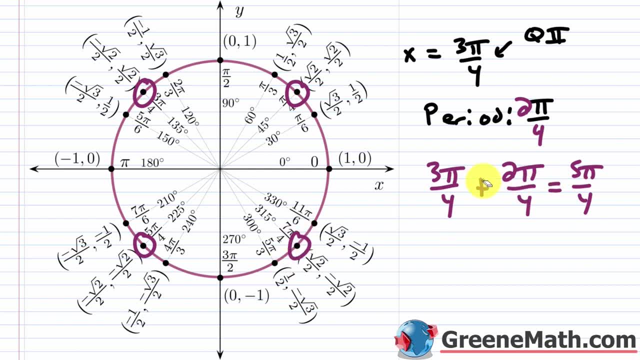 And then in quadrant four, of course it's going to be seven pi over four. But let's just go through it. We would have the five pi over four- this guy right here- And we're adding our pi over two, or two pi over four. 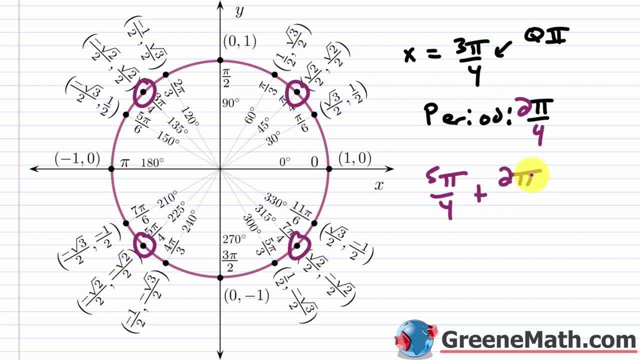 So we have five pi over four plus two pi over four, So that's seven pi over four. So those are your solutions in that interval that I gave. If we have X being greater than or equal to zero and less than two pi, Then X is going to be equal to pi over four. 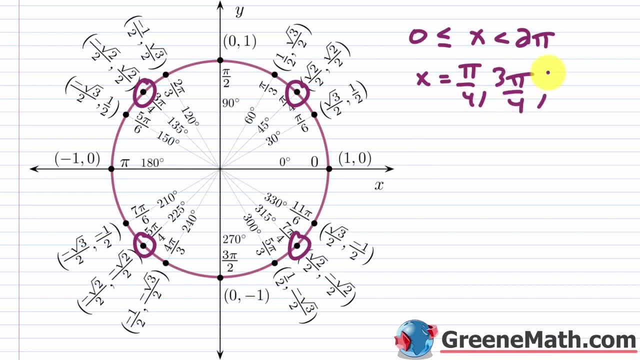 And then you have three pi over four, and then you have five pi over four- Let me scooch this down a little bit- And then you have seven pi over four. Then, in terms of the general solution, if you did want that- although it didn't ask for it- you could start with pi over. 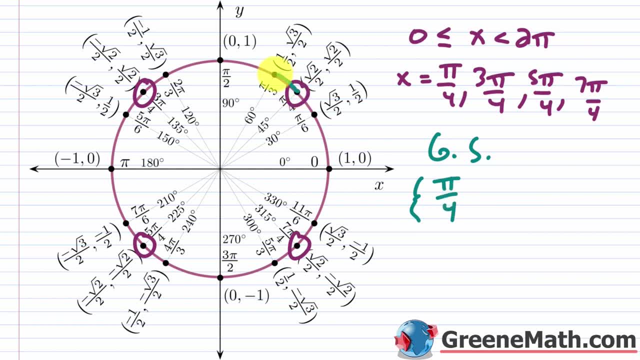 four. So start with something like pi over four, And then you could just add pi over two to get to the next solution, and then add pi over two to get to the next solution, and then add pi over two to get to the next solution, and add pi over two to get to the next solution, And that will continue forever. 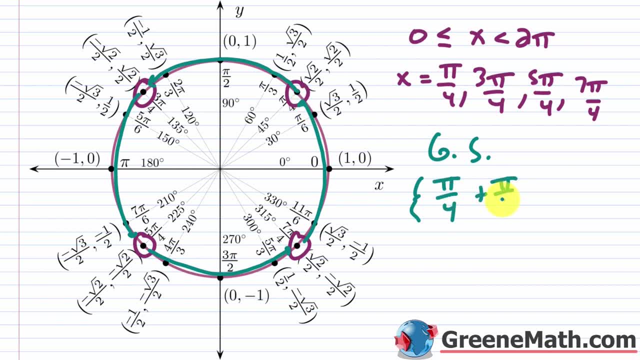 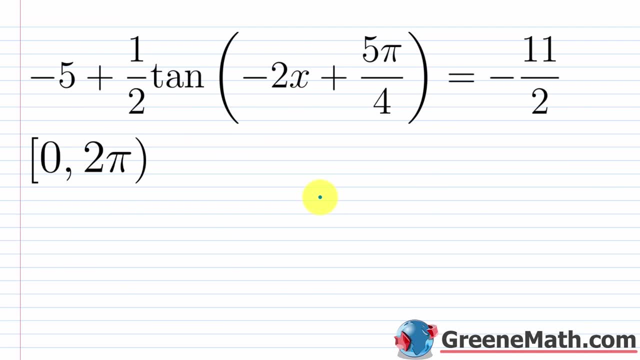 and ever and ever. So pi over four plus your pi over two times n, where n is any integer. All right, one thing that I find helpful, especially for beginner students, is to look at a graph of an equation after you solve it, So you can go to Desmos. So I would say that you have one half. 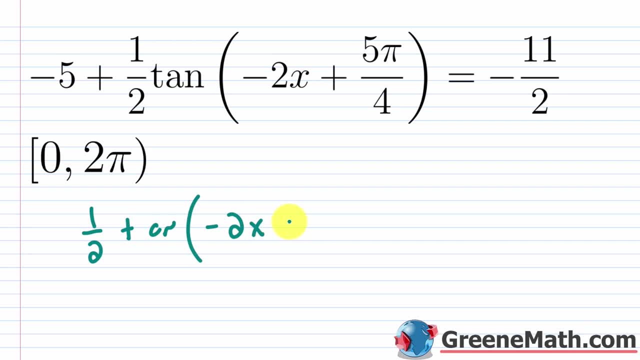 and then tangent of negative two x plus five, pi over four, And then you have this negative five here. So let me write minus five. I'm going to add this to both sides, So I'm going to add 11 halves over here, And then this would be equal to zero, because I added it over here as well. So this: 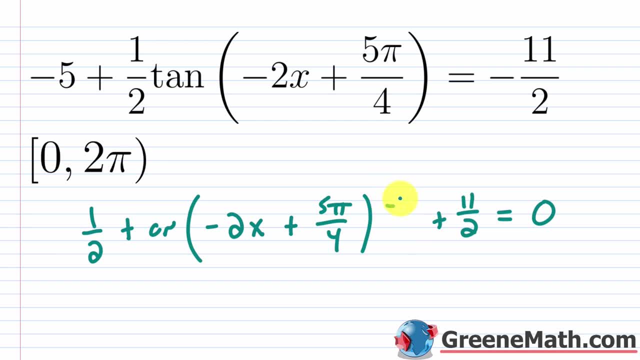 right here, this negative five, that's negative 10 over two. So this is negative 10 over two, and negative 10 plus 11 is going to be positive one. So this right here would be plus one half. So the way you would key this into Desmos is you would say that y is equal to this And, of course, 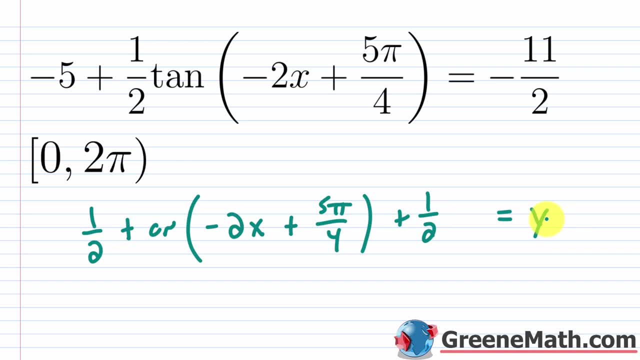 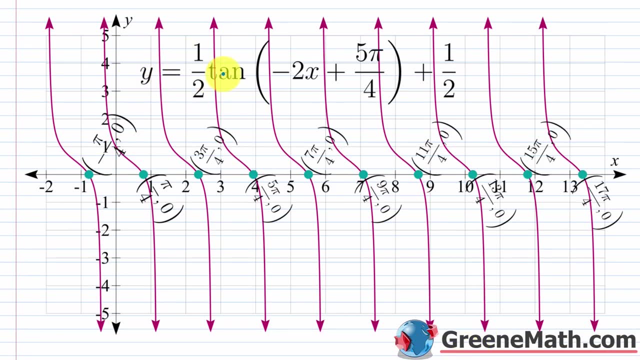 if I plug in a zero for y now I'm just finding my x inverse Or the x values that make the y value zero. So I have the graph set up for us Again. this is: y equals one half tangent of negative two x plus five, pi over four plus one half. So if you 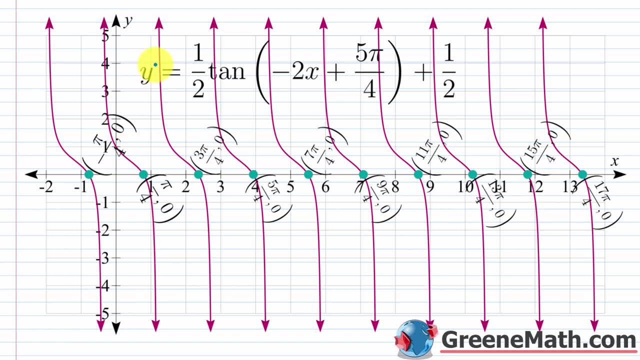 want to key that into Desmos again. if I plugged in a zero for y, now I'm looking for the x intercepts. So where are the x values that make the y value zero? And of course you're going to see, this is consistent with what we found. So here you have, your pi over four, your three pi over. 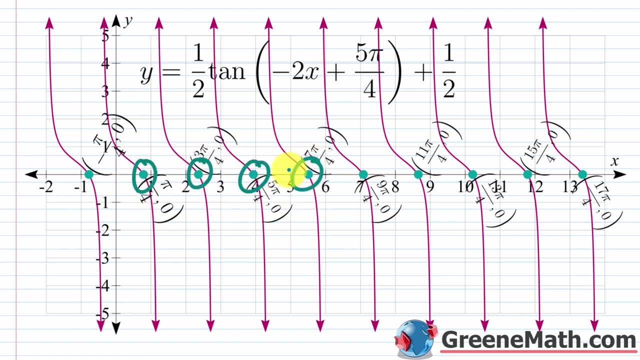 four, your five pi over four, your seven pi over four. So that's in the interval that we solved in, from zero to two pi, where zero is included and two pi is excluded, And then you would continue with this pattern forever, So you can keep just adding pi over two to your solution. 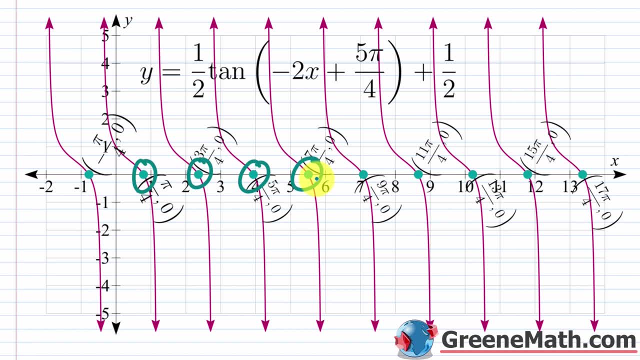 to get to the next one. So seven pi over four plus pi over two, or you could say two pi over four, that's nine pi over four, then 11 pi over four, then 13 pi over four, then 15 pi over four. 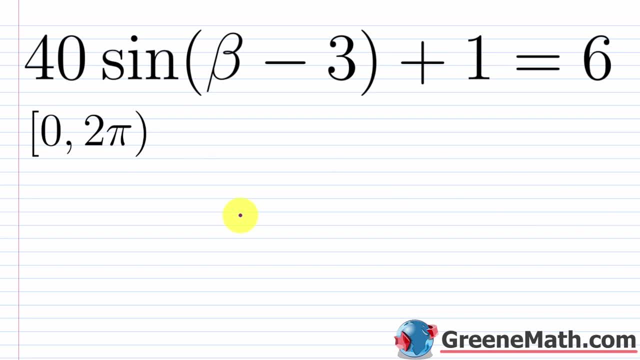 then 17 pi over four, so on and so forth. All right, let's go ahead and look at another example. So here we have 40 sine of beta minus three, then plus one is equal to six. Again we want to solve. 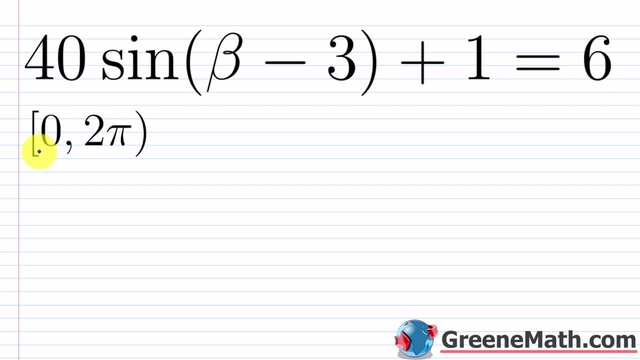 this over the interval from zero to two pi, where zero is included and two pi is excluded. So we're going to have 40 and then sine of this, beta minus three, and then plus one is equal to six. So let me go ahead and grab this. let's come down to a fresh sheet here And again. my goal to start is: 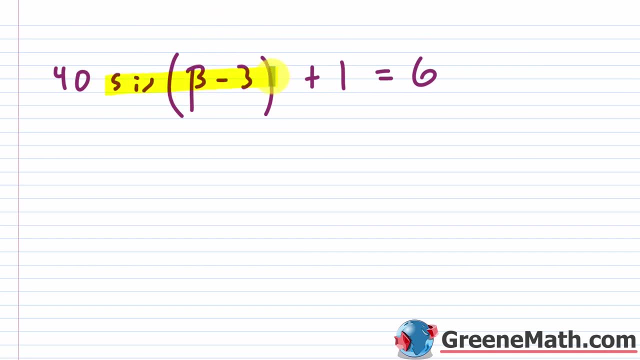 to get the sine of this beta minus three on one side by itself. So I want to isolate that. So, in order to do that, I'm going to start by subtracting one away from each side of the equation, So this and so now we're going to have 40. And I'm going to put times the sine of this beta minus three. 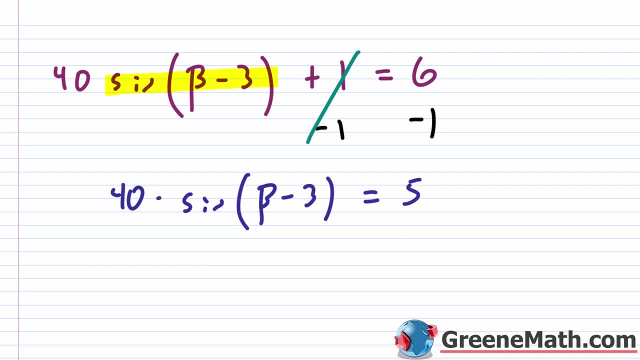 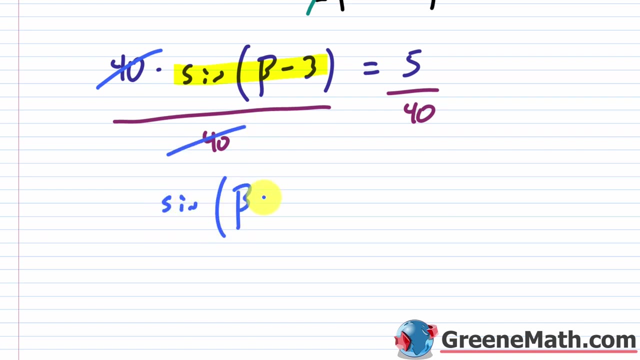 and this would be equal to six minus one is five. Again, I want to isolate this right here. So you have 40. that's multiplying that. So all I'm going to do is divide both sides of the equation by 40. So of course this is going to cancel, And now you're going to have the sine of this beta minus. 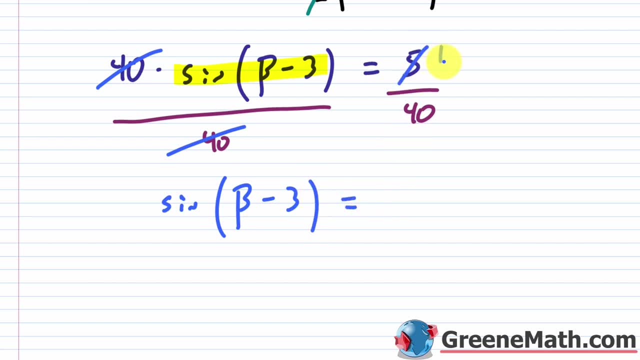 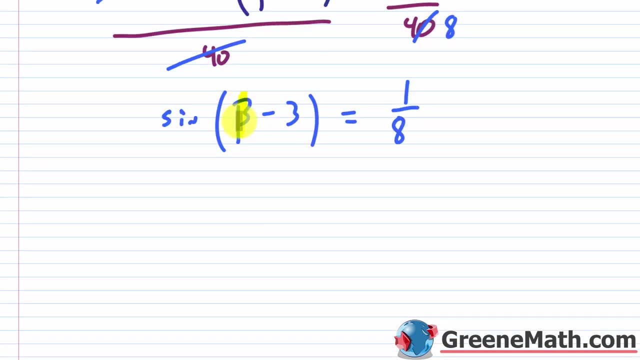 three is equal to when you think about five. divided by five, that's one, and 40, divided by five is eight. So this is one eighth. Now I've got to get this guy by itself, And in order to do that, I've got to get rid of this guy right here. So I'm going to use my property from: 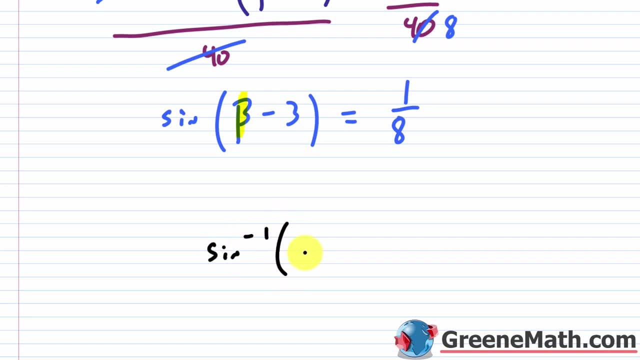 earlier. remember that if you have the inverse sine, so the inverse sine of the sine of x, this equals x as long as x is within the domain of the restricted sine function. So we would say for x being greater than or equal to negative pi over two and less than or equal to pi over two. 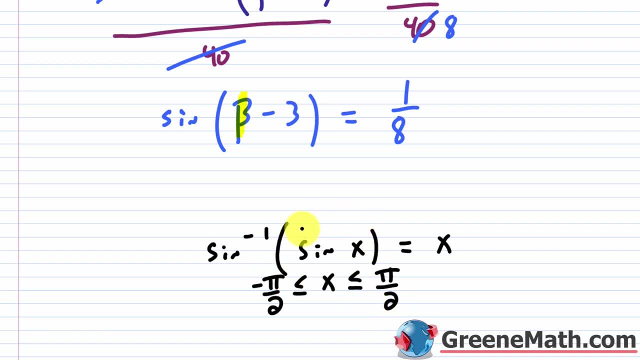 So here I'm just going to take the inverse sine of each side of the equation and I'm going to use this rule here. So let me actually get rid of this And I'm going to say that I have the inverse sine of this guy right here, So the sine of my beta minus three, and this equals. again I'm going 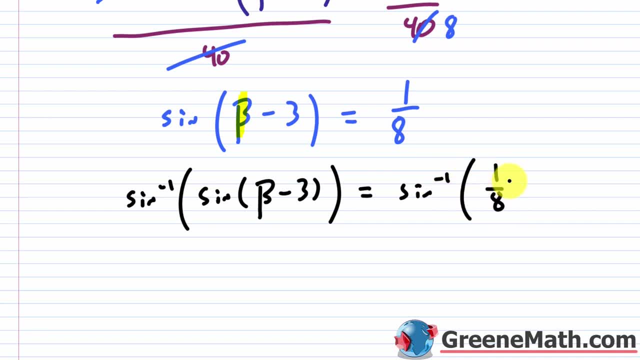 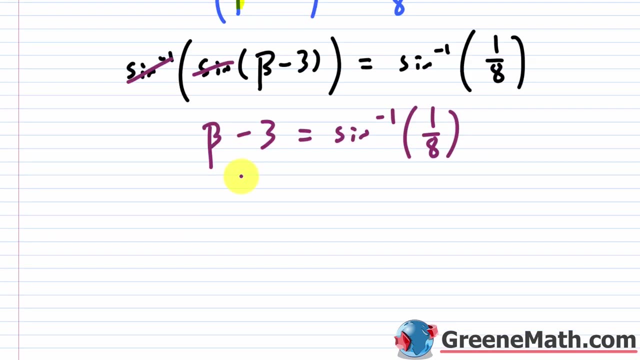 to do that over here as well. So the inverse sine of one eighth. So at this point we know that this will undo this, So those are going to cancel and I'm left with my beta minus three And this equals my inverse sine. So my inverse sine of one eighth. Now, at this point you can give one solution for. 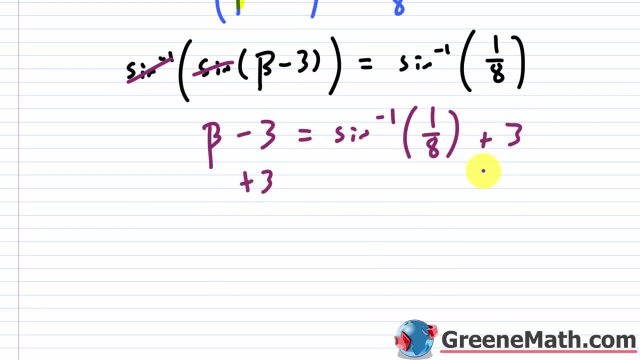 beta. you could just add three to both sides of the equation, And so this right here is going to cancel, And you're going to say that beta is equal to the inverse sine of one eighth and then plus three. So this is only one solution. To get the other solution, what you're going to have to do, 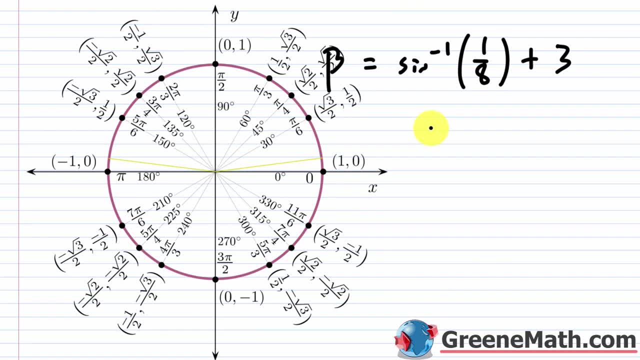 is think about your angle. in quadrant two that has a sine value of one eighth. So what do I mean by that? Remember that if you have the inverse sine of something that's positive, so this is a sine, and then plus three, this is a sine. So what you're going to do is you're going to get this. 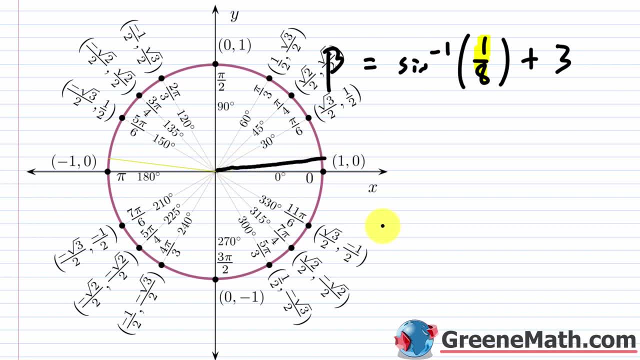 angle right here. let me try to trace over this as best as I can. So that angle right there, if you're working with radians, that's going to be. let me put: the inverse sine of one eighth is about 0.125.. 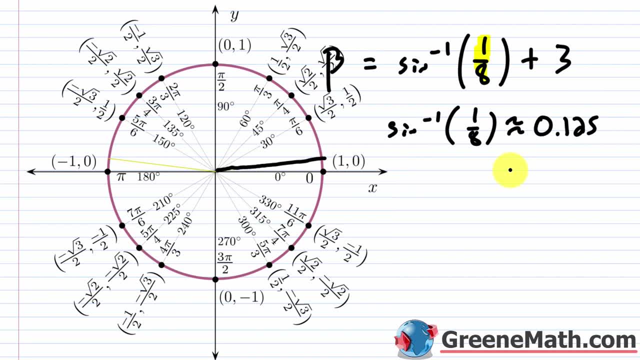 In terms of radians. if you want to work with degrees, it would be about 7.18 degrees. So that's going to be for that angle, right there. Let me just put this in so everybody knows what that is. So this is going to be about 7.18 degrees. 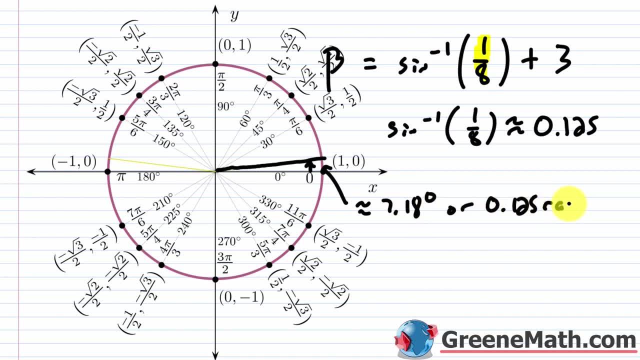 Or 0.125 radians. Now, where is the sine value also going to be one eighth? Well, again in quadrant two, where I have a reference angle of 7.18 degrees, or 0.125 radians. So you want. 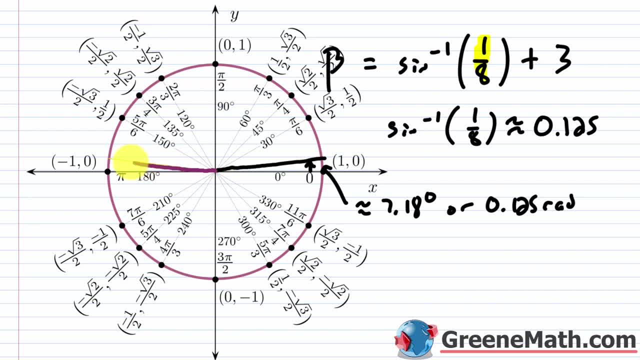 this angle right here as well. So this angle right here as well, which again would have that same reference angle. So if I go down like this, this would be about about 7.18 degrees or 0.125 radians. Now how do I get this angle right here? So this is the angle if I look at it. 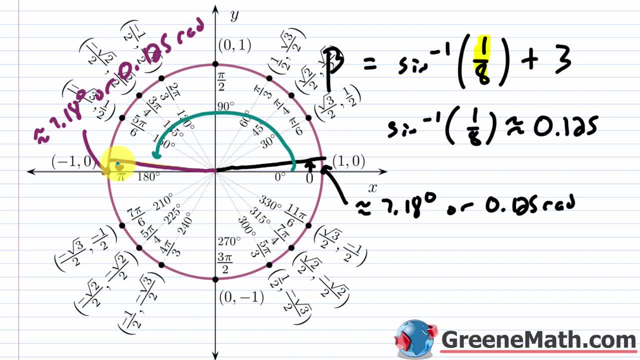 well, all I have to do is take the straight angle, which is pi, and subtract away this part right here. So you could do that by saying that you have. your beta is equal to pi minus the inverse sine of one eighth. So again, that's taking this piece out, and then plus three, like that. So let me go. 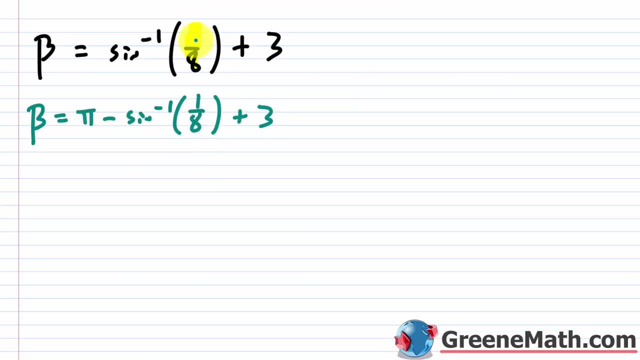 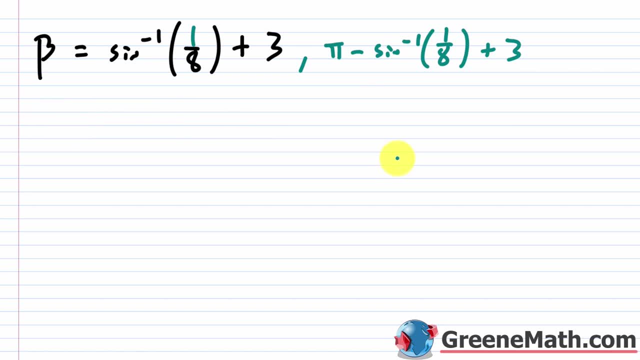 I'll just put a comma here. you can also use solution set notation if you want. Now, if you wanted to give the general solution, then basically all you'd have to do is say: this guy plus two pi n or n is any integer. and then this guy plus two pi n or n is any integer, because your solutions 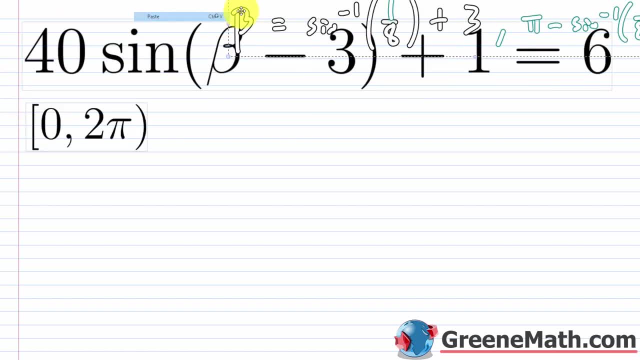 are going to repeat every two pi. Now, if you want, let me go ahead and grab this real quick. Let me paste this in: If you want to verify these solutions again, you can sketch the graph of this guy. The way I would do it is, I would say that: 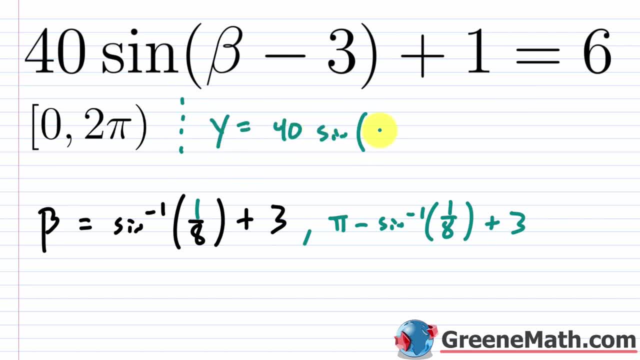 you have, y is equal to 40 sine of beta minus three. and then I would subtract six away from each side, So I would say minus five. So basically, if you subtract six away from each side here you would have this part right here is equal to zero. I'm replacing the zero with y, So I can. 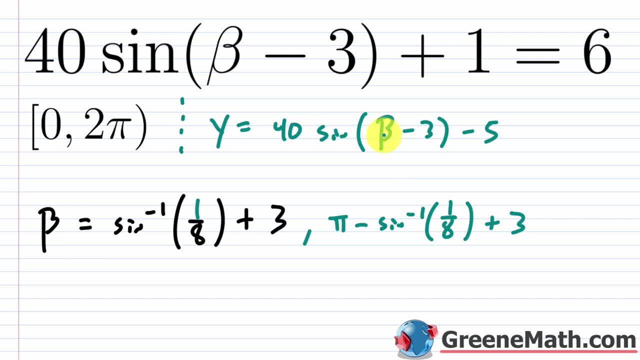 graph this guy. And again, if y is zero, you're looking for the value for beta. or you could put an x here, if you want, for graphing purposes. So you're looking for the value for x, such that the y value is zero. So you're looking for the x intercept. 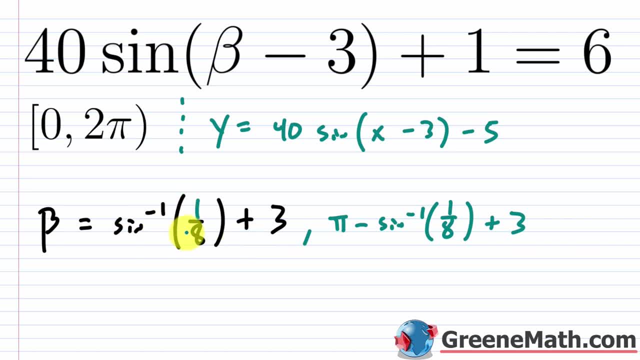 Now, in terms of approximating this again, the inverse sine of one eighth, that's going to be about 0.125.. And then if you add three to that you're going to get about 3.125.. So let's say that. 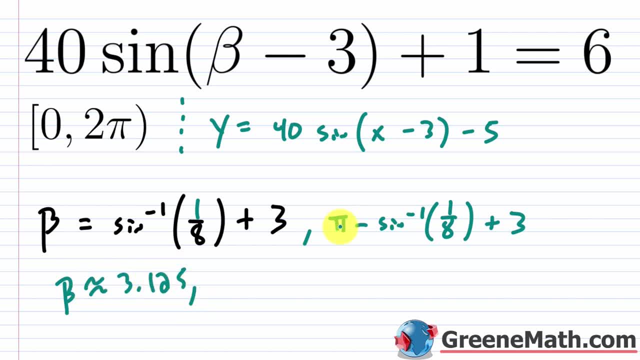 beta is about 3.125.. So if you key this into your calculator you're going to get about 6.01.. Let's just say six, So 6.016.. Like that. Let me just grab this real quick. So, coming down to the graph, 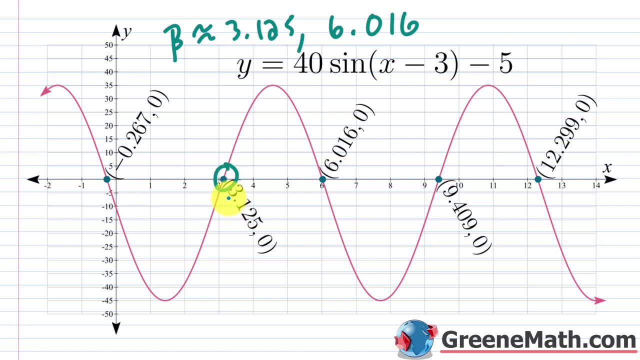 again. you can sketch this on Desmos. This is one of the solutions we found, So about 3.125.. This is another one, So this is about 6.016.. So that's all in the interval from zero to two pi. 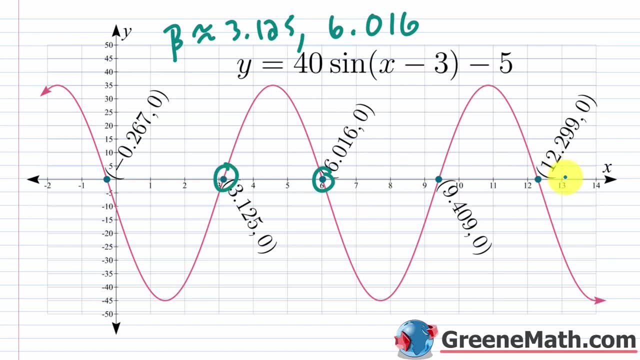 where zero is included and two pi is excluded. And, of course, if you wanted other solutions, if you wanted to give the general solution, everything is going to repeat every two pi. So if you take this solution and you add two pi, you're going to get to this solution here. If you. 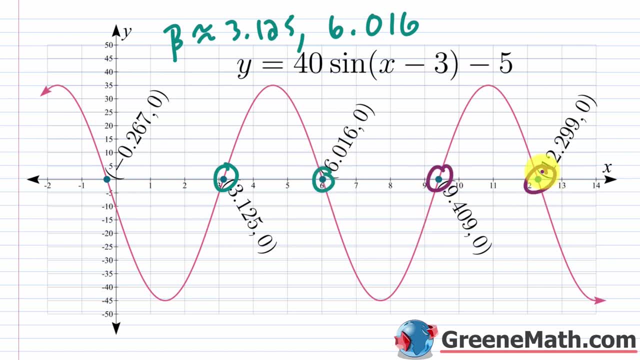 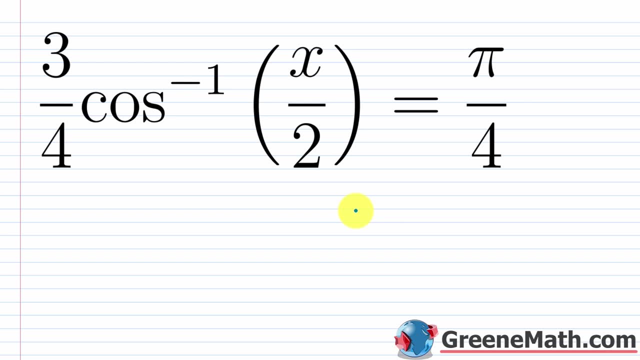 take this solution and you add two pi, you're going to get to this solution here. All right, let's change things up, And now we're going to look at some problems that involve solving equations where you have an inverse trigonometric function involved. So here we have three fourths. 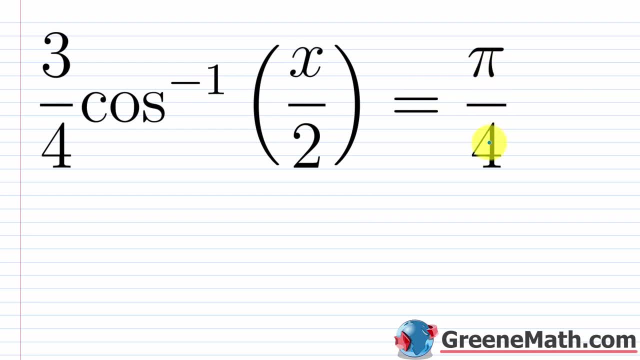 times the inverse cosine of x over two. And then we're going to look at some problems that involve. this equals pi over four. Now, for this type of problem, what you want to do is isolate your inverse cosine function. So I want inverse cosine of, in this case, x over two on one side. 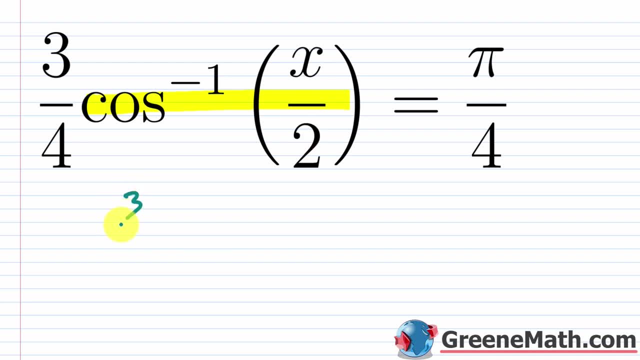 and I want a number on the other. So let's go ahead and just copy the problem. So three fourths- I'm going to put times the inverse cosine of this, x over two, and this equals pi over four. If I want to isolate this guy right here, we'll have three fourths. that's multiplying this guy. 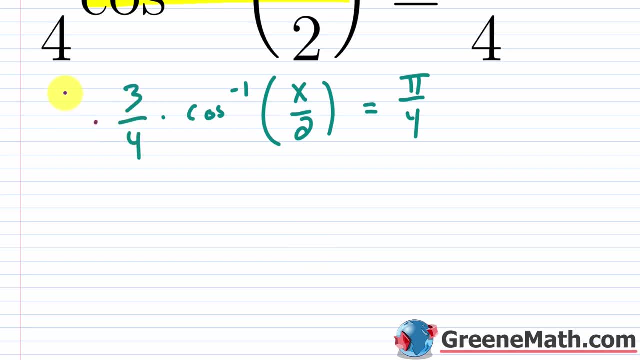 So what I'm going to do is multiply both sides of the equation by the reciprocal of three fourths, which is four. Remember that a number times this reciprocal will always give you one. So when I multiply four thirds times three fourths, those guys are going to cancel and give me a big fat one. 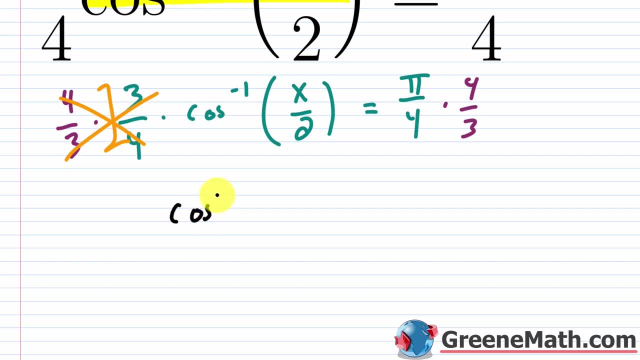 So now the left side is just what I want. It's the inverse cosine of this: x over two And this is equal to over here. the fours would cancel, And so you would have pi over three. Now, at this point you could probably solve this by inspection. you can just look at this and say: well, 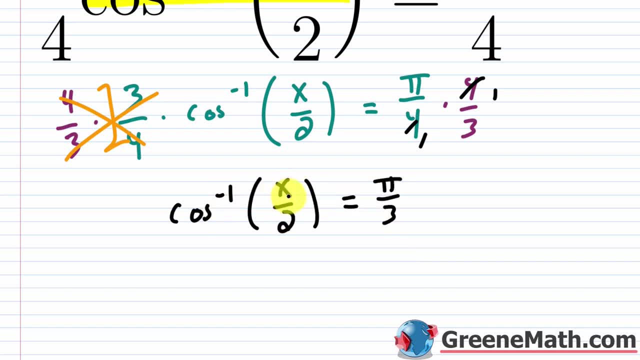 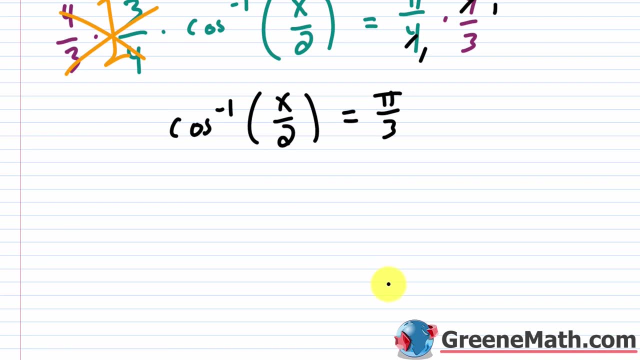 the inverse cosine of one half would be pi over three. So I know x is going to end up being one. It's a really easy equation. But if you didn't know that, what could you do to get your solution? Well, there's two strategies you could use. The first thing is you can go back to what we talked. 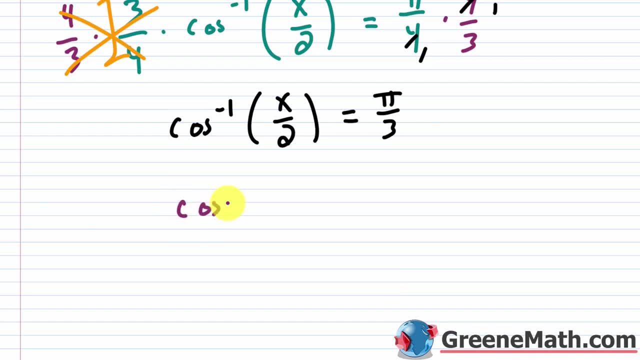 about earlier with the cancellation property. So if you have something like the cosine of, the inverse cosine of, let's just say x- right now we have x over two, but let's just say x- this would be equal to x as long as this guy is within the domain of the inverse cosine function. 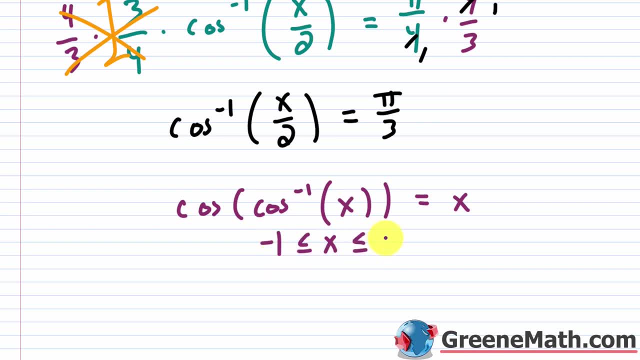 So as long as x is greater than or equal to negative one and less than or equal to positive one, Now we're just going to use that to solve this problem. So let's just say x is greater than negative one. So let's just say x is greater than negative one, And then I'll show you an easier. 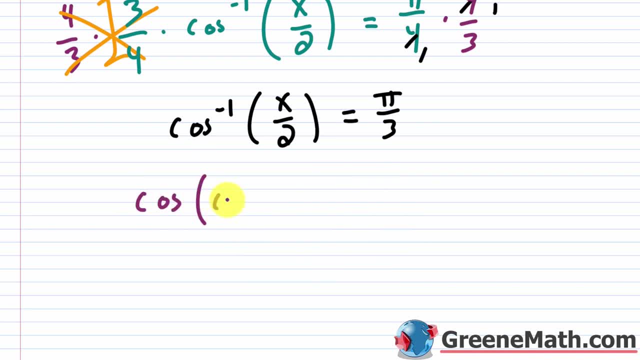 way to do it. So I'm going to take the cosine of each side, So the cosine of the inverse cosine of x over two is equal to. I'm going to take the cosine of this side as well, So the cosine of pi over three. So at this point I'm just going to cancel this with this. these guys will undo each. 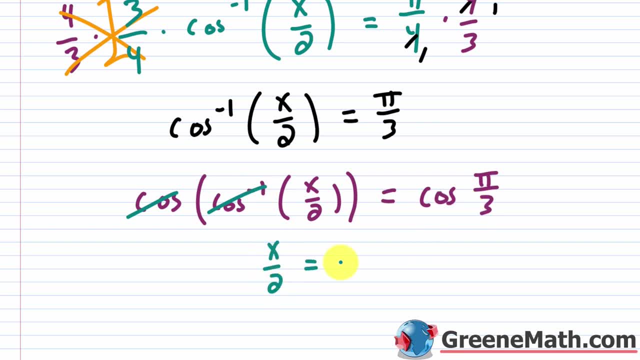 other and you're going to have: x over two is equal to the cosine of pi over three, we know, is one half, And at this point you know that x is one. right, the denominators are equal. So you could, if you wanted, to just multiply both sides by two. let's just go ahead and clear the. 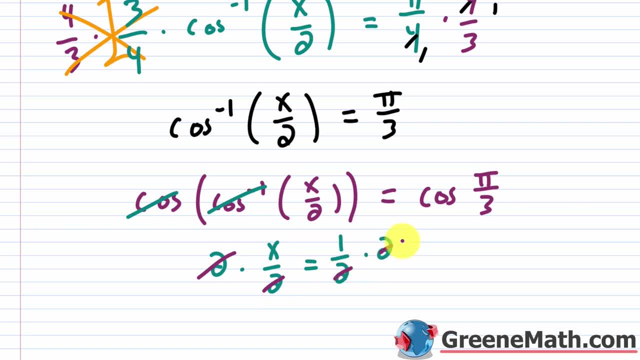 denominators away to make this official. So this guy, we cancel with this guy. this guy, we cancel with this guy, and you get x is equal to one. An alternative approach, if you get something like this- let me get rid of this right here- is to do this in a simpler way. So you'll probably. 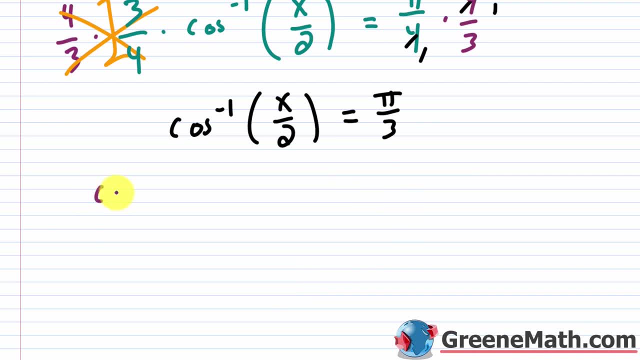 see this technique in your textbook. you know that if you have the cosine of pi over three, you get one half. So this is the angle, this is the cosine value. then you also know that the inverse cosine of one half- so that's the cosine value- this is going to give you the cosine of 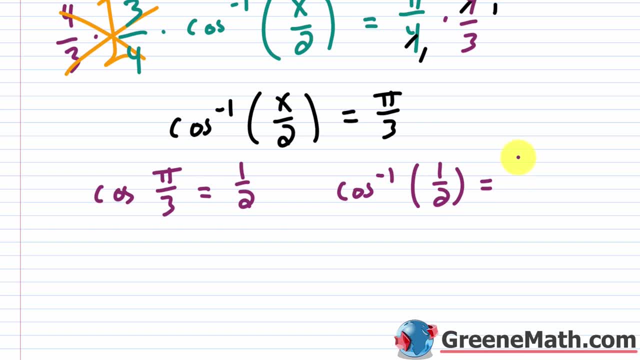 you the angle again between zero and pi, where zero and pi are both included where that cosine value is one half. So this is pi over three. So if I look at this, the inverse cosine of x over two is equal to pi over three. well, this is your cosine value And this is the angle. So all I 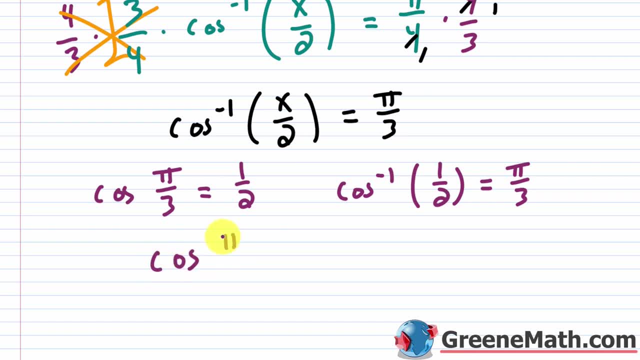 really have to do is say: well, that means that the cosine of the angle pi over three is equal to- again, this is the cosine value, So this is x over two. So you can kind of shortcut that process and just set it up this way, just using the basic definition for cosine and inverse. 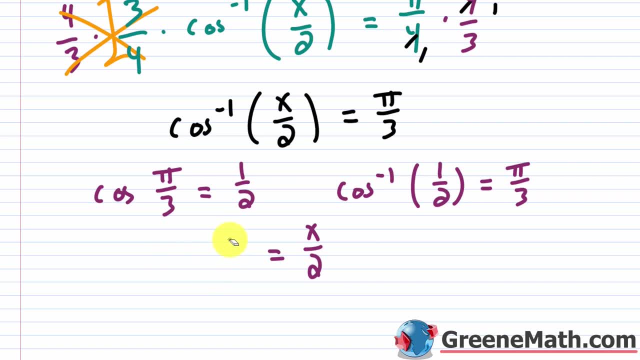 cosine. So once I look at this, I know that the cosine of pi over three is again one half. So this becomes one: half is equal to x over two And that just becomes x is equal to one. Now, with these problems, I always suggest checking them. you'll get a lot of problems that they throw at. 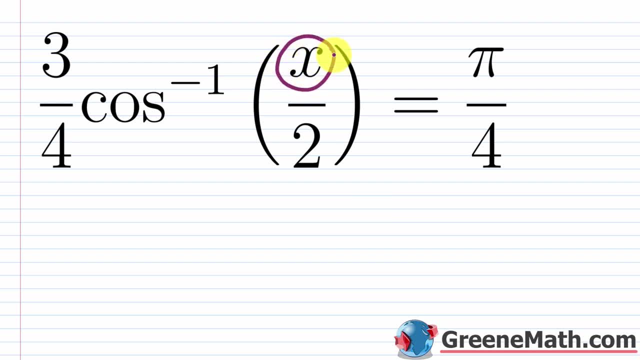 you with no solution here or they get really tricky. So always check your problems here. So what I would do is plug in a one for x and see if I get a true statement. So you get three fourths times. the inverse cosine of one half is that equal to pi over four. So the inverse cosine of 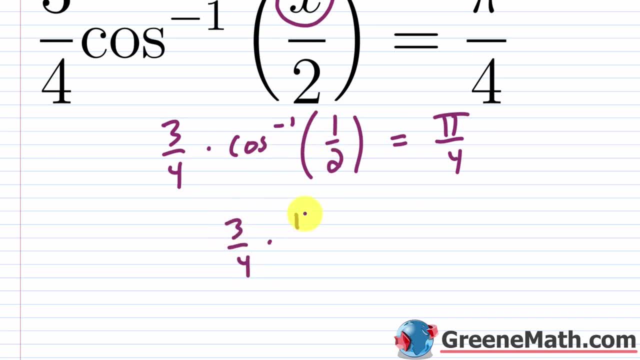 is going to be pi over three, So you would have three fourths times pi over three. Is that equal to pi over four? Yes, it is. If you cancel this with this, you would have pi over four is equal to pi over four. So x equals one is a valid solution, Alright. so again, I'm going to 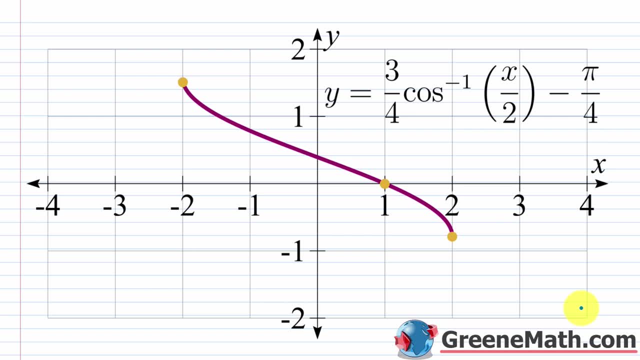 recommend that in this particular section you look at the graph of everything, just so you can confirm things. So I went ahead and just rearrange the equation So I could get y equals three, fourths times the inverse cosine of x over two, and then minus pi over four. So I'm going to 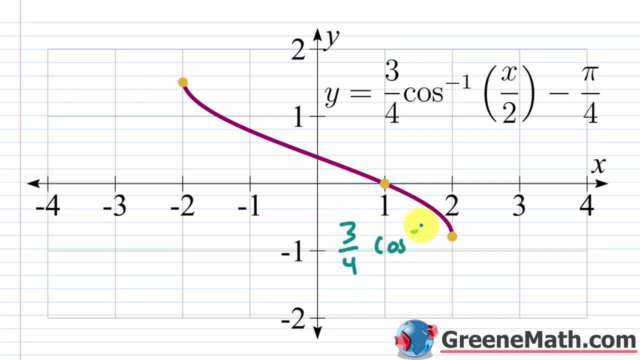 get y equals three fourths times the inverse cosine of x over two, and then minus pi over four. So the equation was three fourths and then cosine inverse of x over two and that was equal to pi over four. So I just subtracted pi over four away from each side, So that would give you minus pi over four. 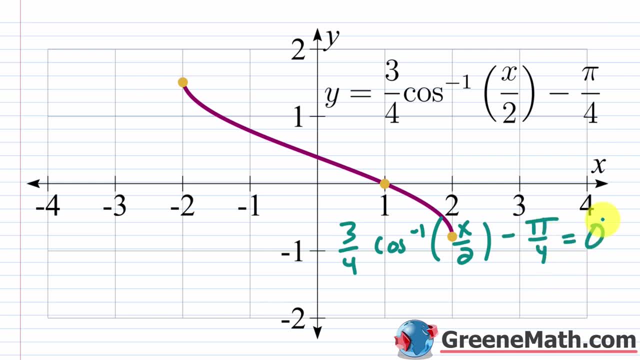 like this, And that would be equal to zero. So again, all I'm doing is I'm plugging in a zero for y And I'm saying: for which x value am I going to get a y value of zero? So where's the x? 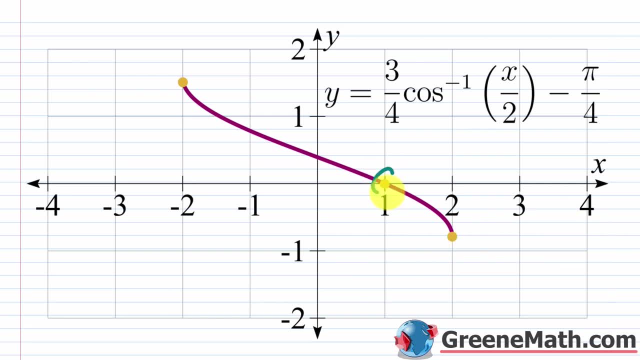 intercept. If you look at the graph where you're going to see, that occurs right here, where you have a one for your x value and a zero for your y value. So the ordered pair: one comma zero, And that confirms our solution: that x is going to be equal to one. All right, let's take a look at. 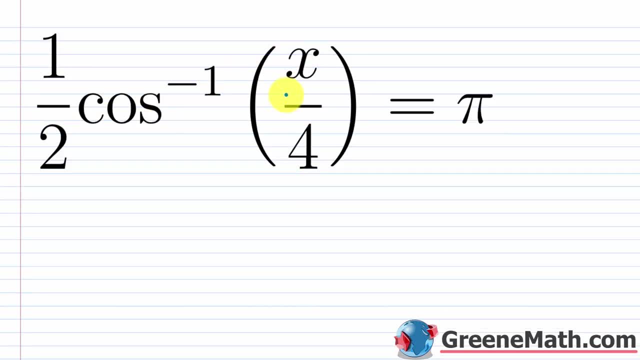 another one. So here we have one half times the inverse cosine of x over four. this is equal to pi. So in this particular case again I'm trying to isolate the inverse cosine function first. So here the inverse cosine of x over four. So let me just write: one half times the inverse cosine. 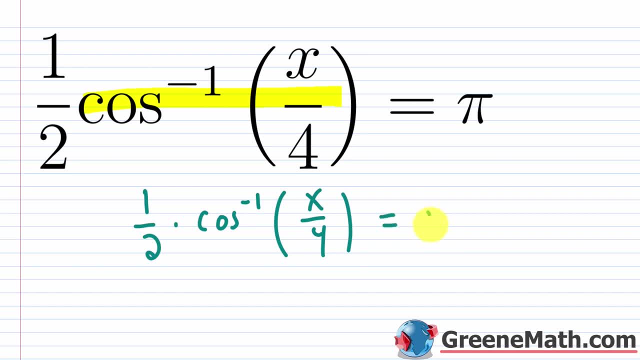 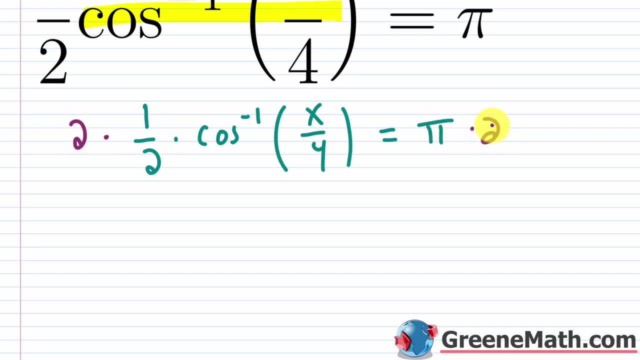 of x over four, And this would be equal to pi. Now, if I want to isolate this guy, I need to get rid of this one half that's multiplying it. So I'm just going to multiply both sides by two, And so we're going to see that this right here is going to cancel with this right. 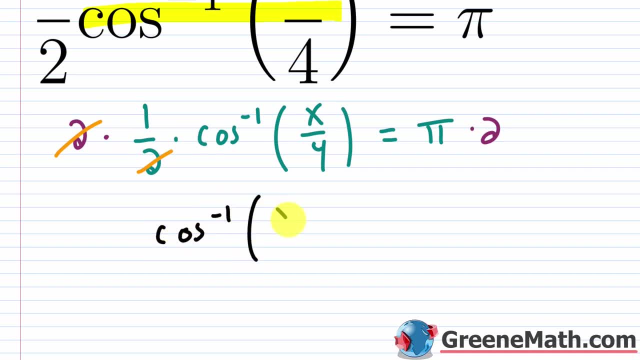 here. So now I have my inverse cosine of x over four. that's on the left, it's isolated And this equals pi times two is just two pi. Now let's stop for a moment and think about this. Is there going to be a solution for x? Is there something that I can plug in there? divide by four and then take. 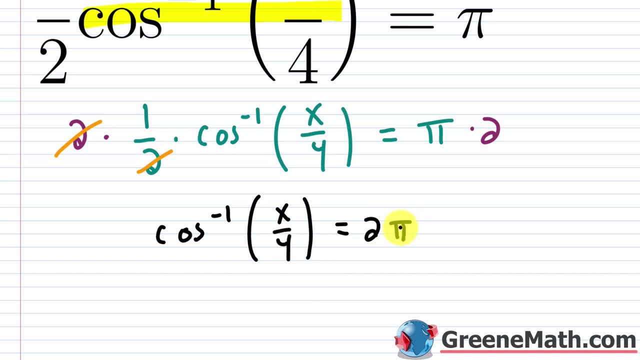 the inverse cosine of that and get two pi. No, because the range of the inverse cosine function is from zero to pi, with zero and pi both being included. This right here is impossible. So we would say that there's no solution, right? So there's no. 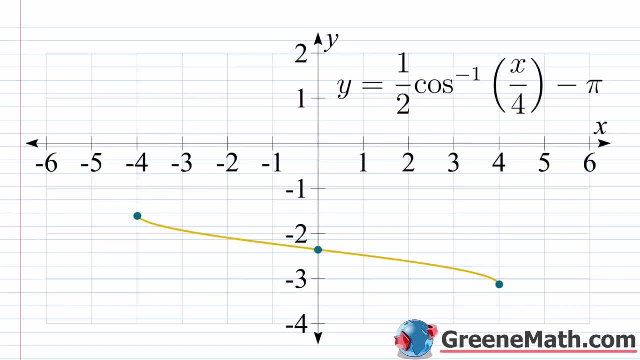 solution. Again, if you want to look at this graphically, if you started with one half times the inverse cosine of x over four, and again, this was equal to pi. So let's put equals pi. Well, I'm going to subtract pi away from each side, So now I'll have minus pi equals zero. Well, 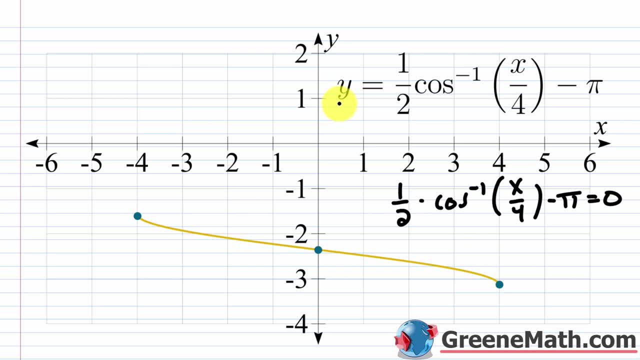 again, I'm just plugging in a zero for y And I'm saying: for which x value am I going to get a y value of zero? So where would I cross the x axis or get an x intercept? And you can see that this graph does not cross the x axis. Basically it goes from here to here. 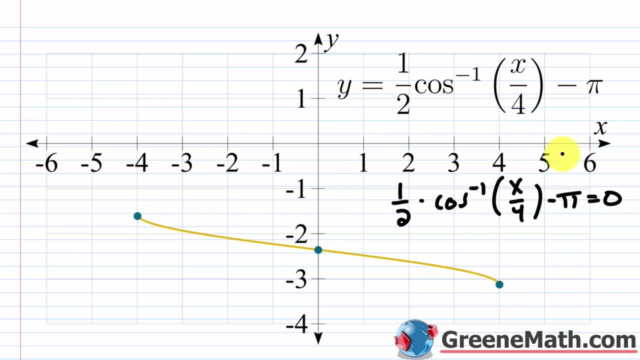 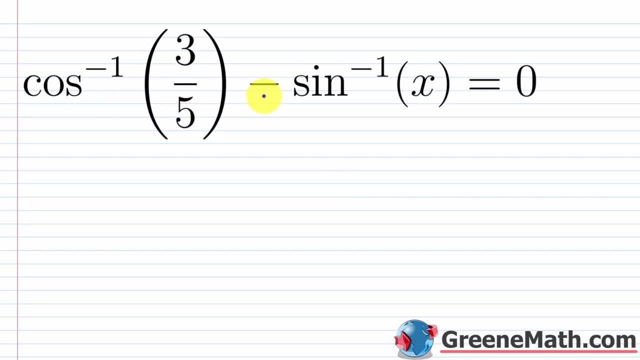 It's never going to cross the x axis, So there is no solution. All right, let's take a look at a problem that's a little bit more tedious. So here we have the inverse cosine of three fifths minus the inverse sine of x, and this equals zero. So if you get a problem like this, what I would do is I: 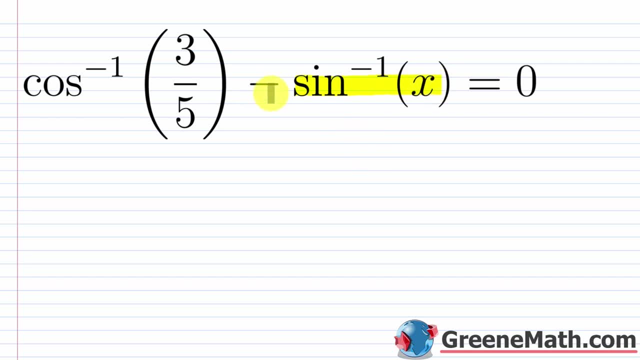 would isolate the inverse sine of x. So in other words, right now you have minus the inverse sine of x, So I would add the inverse sine of x to both sides. So let me just show that real quick. So I'm going to add the inverse sine of x on the left And I'm 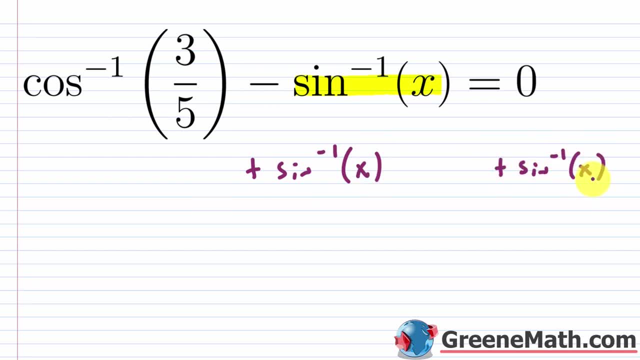 also going to add the inverse sine of x on the right, So this would cancel away. So what I would have here is the inverse cosine of three fifths is equal to the inverse sine of x. So I'm actually going to write this one on the left. That's just my preference. So I'm going to write the inverse. 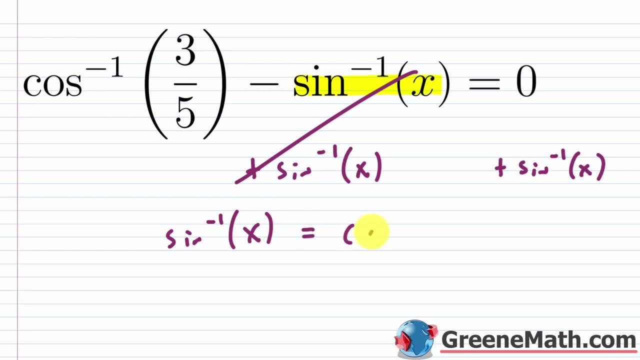 sine of x is equal to the inverse cosine of three. Okay, I'm going to come down to a fresh sheet, So we have a lot of room to work. So what I'm going to do is actually take the sine of each side. So I'm going to say that I have the sine of the 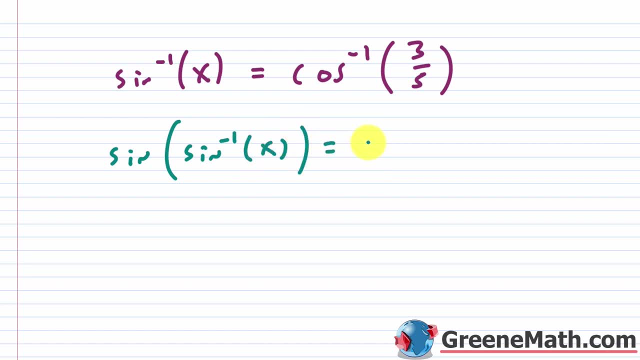 inverse sine of x And this equals- I'm going to take the sine of the inverse cosine of three fifths When I think about taking the sine of, again, the inverse sine of x. these guys will undo each other as long as x is within the domain of the inverse sine of x. So I'm going to take the. 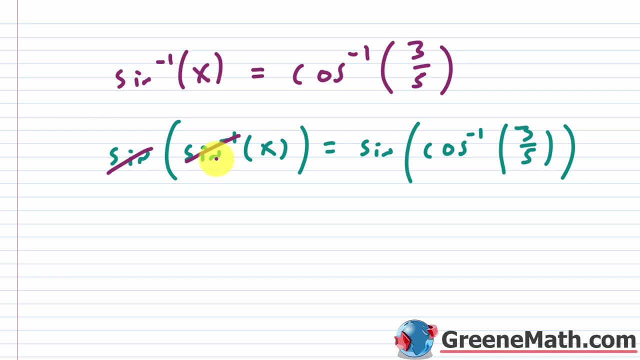 inverse sine function. So from negative one to positive one, with both being included. So x is equal to the sine of the inverse cosine of three fifths. What is the inverse cosine of three fifths? Again, that's an angle in quadrant one, because this guy is positive where the cosine value is. 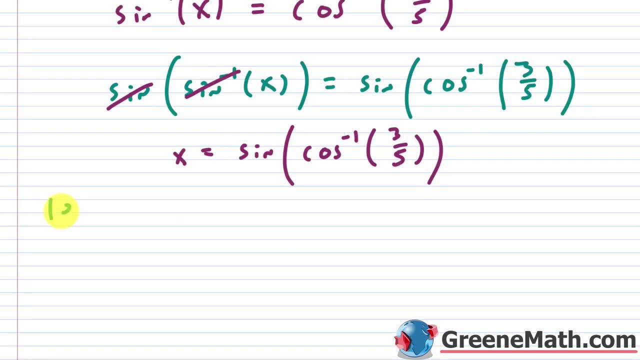 going to be three fifths. So what I can do is say that I'm going to let something like theta be equal to the inverse cosine of three fifths. So what I can do is say that I'm going to let something like theta be equal to the inverse cosine of three fifths. So again this angle: theta is going to be. 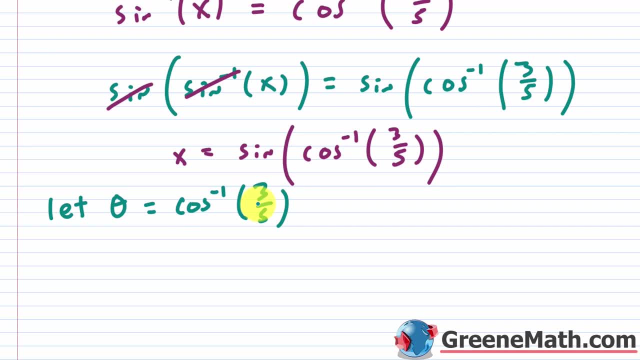 in quadrant one, because the inverse cosine of something that's positive is going to give me something in quadrant one. So I'm going to say that theta is in quadrant one. Additionally, we know that this right here is the cosine value. So I can say then that the cosine of this theta, 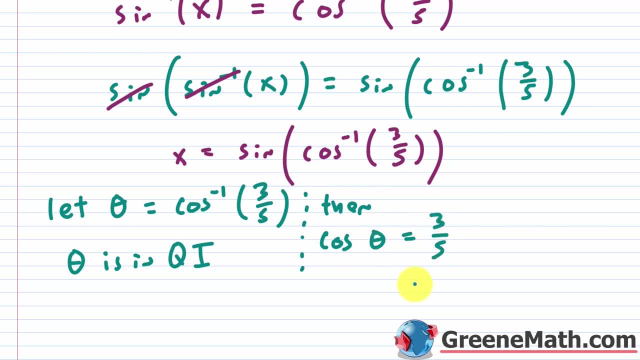 is going to be three fifths. So what am I really trying to find for x here? Well, it's the sine of, again the inverse cosine of three fifths. So I'm going to say that I'm going to let something like: 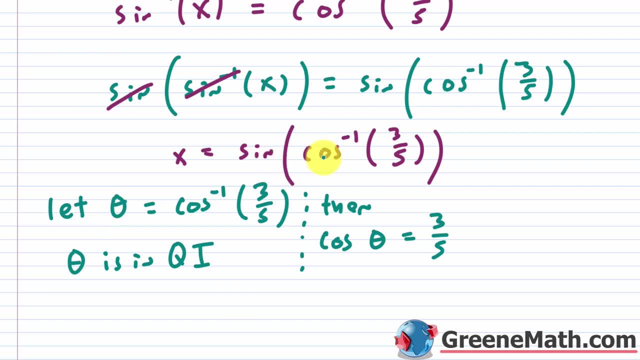 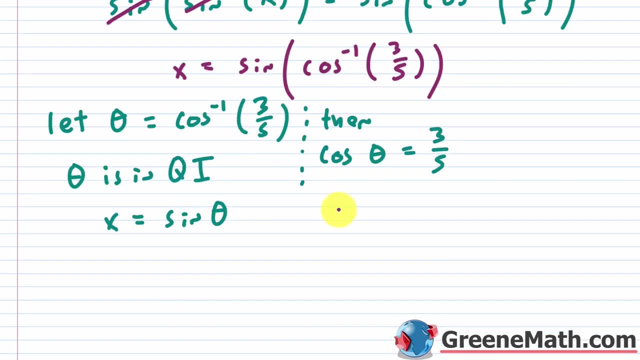 Well, the inverse cosine of three fifths is theta. So really, I'm just trying to find the sine of theta. So you could really write this as x is equal to the sine of theta, How do we figure out what the sine of theta is? Again, if I know, the cosine of theta is three fifths and I know theta is in. 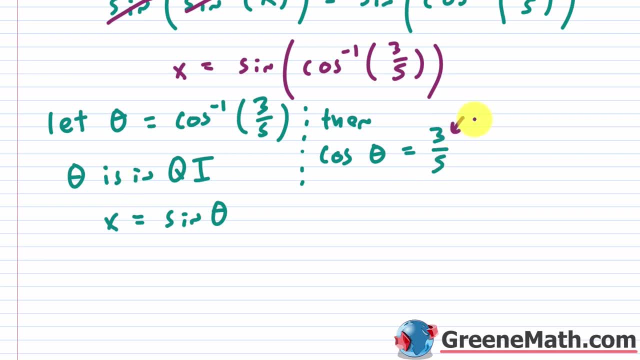 quadrant one. this is really easy to figure out. So this right here is your adjacent And this right here is your hypotenuse. Remember, for cosine it's adjacent over hypotenuse. Again, you could also say that this is your x over your r, For the sine of theta, this is going to be your opposite. 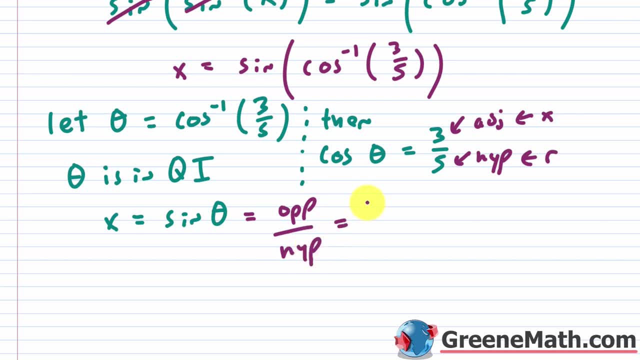 over your hypotenuse, Or you could write that as your y over your r. Well, I know that the r or the hypotenuse in this case is five, So I can just put that in there. And again, you could just use your. 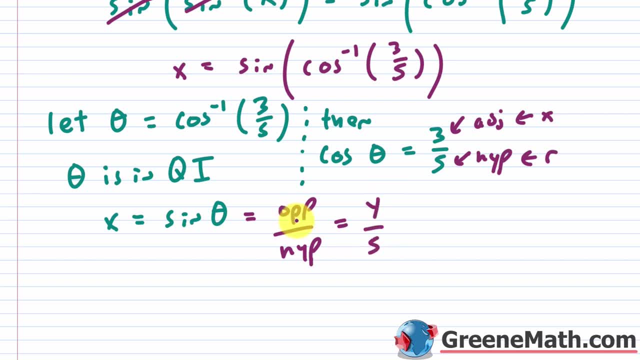 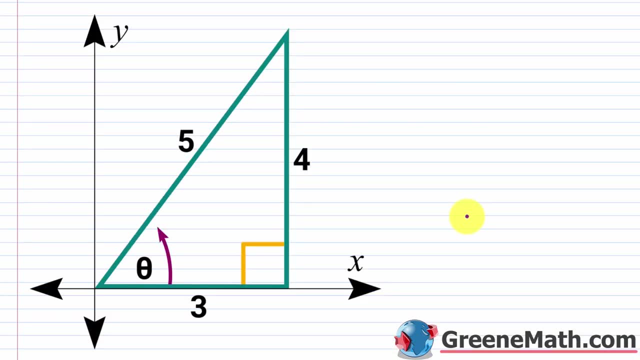 Pythagorean theorem to figure out what y is, or the opposite. A lot of you already know it's going to be four, because this is a three, four, five right triangle. But again, you can always make a sketch. Now for this one it's very easy, So maybe you don't need a sketch. 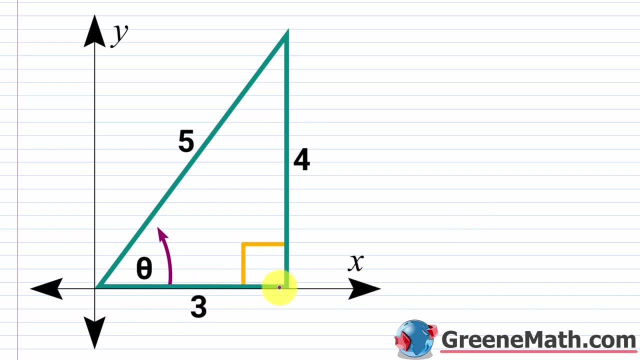 But I'll just go ahead and make one for completeness. So the adjacent is going to be three. So you could say: this is your x here. So x is three, your hypotenuse is going to be five. So I'm going to say: this is your r, r is five, And of course the opposite, or your y is going. 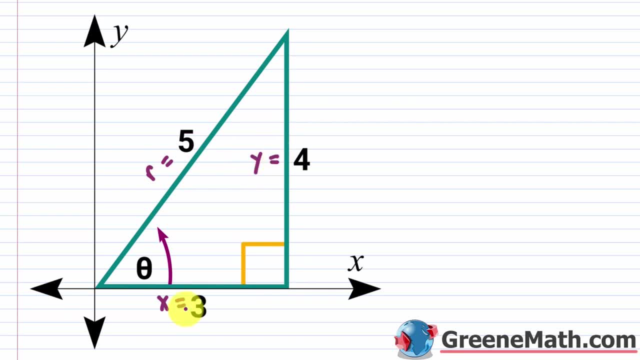 to end up being four. But when we first solve the problem, we don't know that. So what you would do is say that you have x squared plus y squared is equal to r squared, just coming from the Pythagorean theorem, And so we know x is going to be three. So three squared is nine, and then plus. 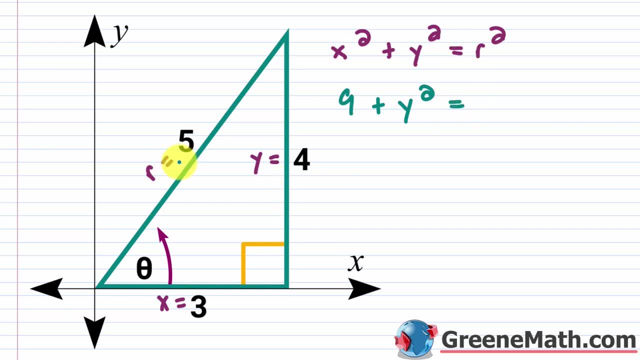 y squared Again. at this point y is unknown And this equals: we know r is five, So five squared is 25.. So what I would do at this point is: subtract nine away from each side of the equation. This cancels, you get: y squared is equal to 25 minus nine is going to be 16.. And at this point, 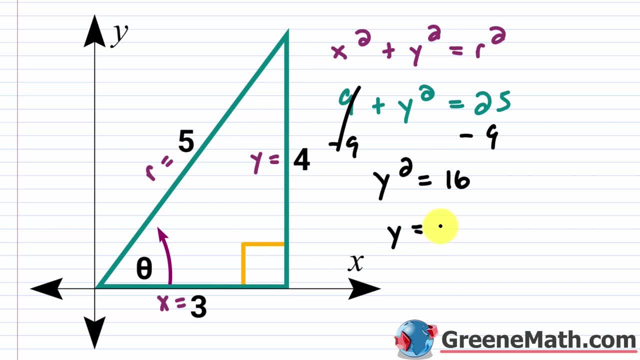 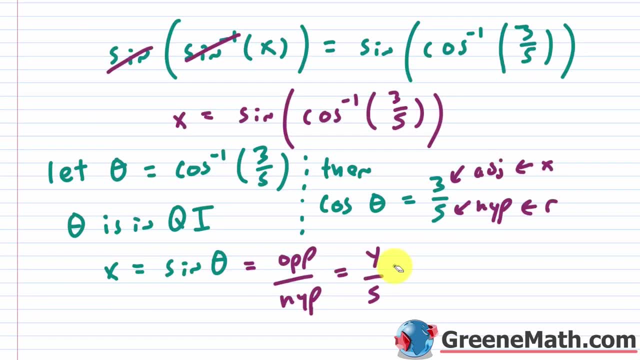 I would say that y is equal to the principal square root of 16,, which is four. you would use the principal square root here because you're in quadrant one and y values are positive. So, coming back here, this would be a four. 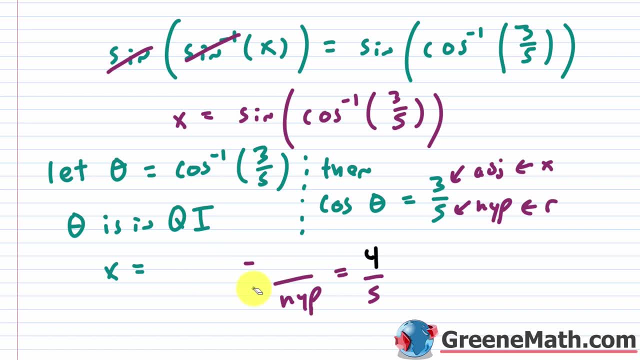 So you can just say that x is going to be equal to four fifths here. Now, how would you check something like this? Remember that theta is an angle whose cosine value is three fifths and whose sine value is four fifths. So, coming back up here again, if you plugged in a four, 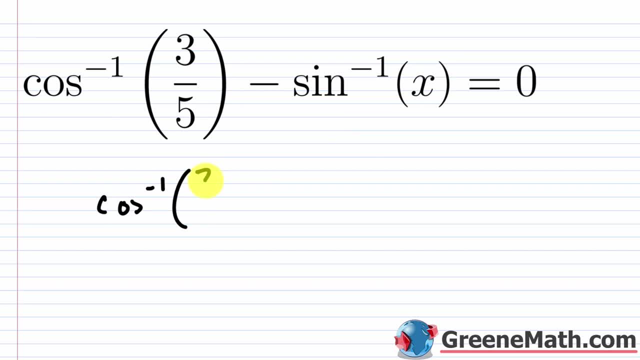 fifths. there you'd have the inverse cosine of three fifths minus the inverse sine of four fifths. Does that equal zero? So essentially, what you have is: let's just say this is theta. Well, this would also be theta. it's the same angle, right? So the cosine of this angle is: 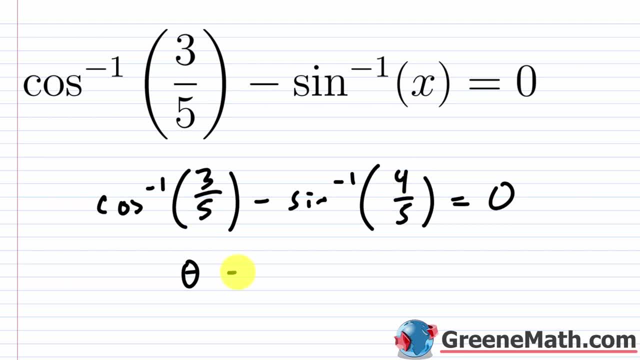 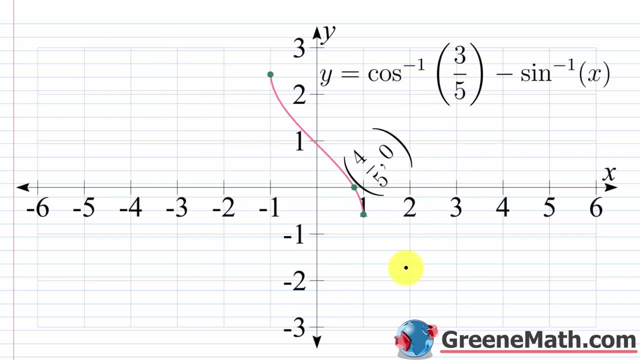 three fifths, and the sine of this angle is four fifths. So it's just theta minus theta is equal to zero. So you get zero equals zero. So this four fifths is a valid solution for x. Again, you can always go to Desmos and verify this solution graphically. So if you do something, 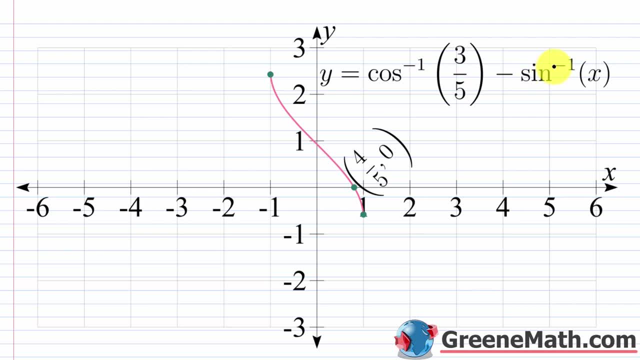 like y equals the inverse cosine of three fifths minus the inverse sine of x. again, if you plugged in a zero for y, you'd have the inverse cosine of three fifths minus the inverse sine of x. I'm asking for which x value? am I going to get a y value of zero? and that's going to occur at four. 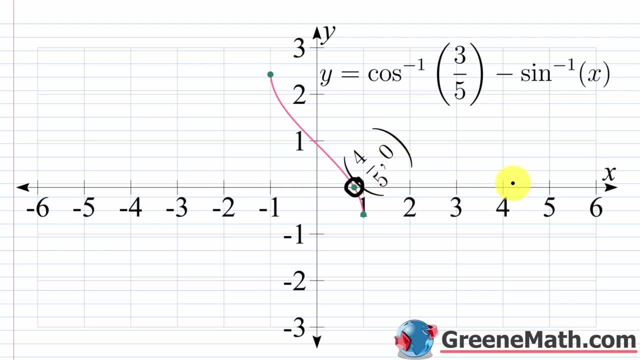 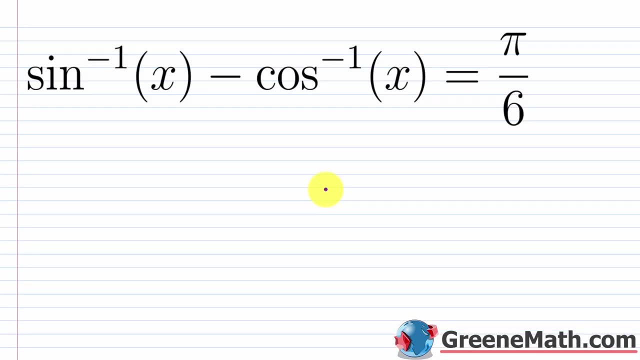 fifths comma zero. So this right here is your x intercept again where y is zero. So that confirms our solution that x is going to be four fifths All right. now let's look at something that's very tedious overall. I'm just going to tell you that you're definitely going to get problems like 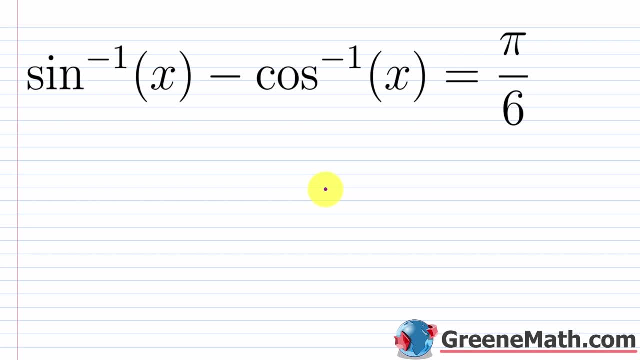 this in your textbook and they take quite a while to solve, especially if you're doing this the long way. I'll also tell you that for most of these problems there's an associated identity that you can use to greatly speed up your work. I would suggest, for the first few times, that you solve: 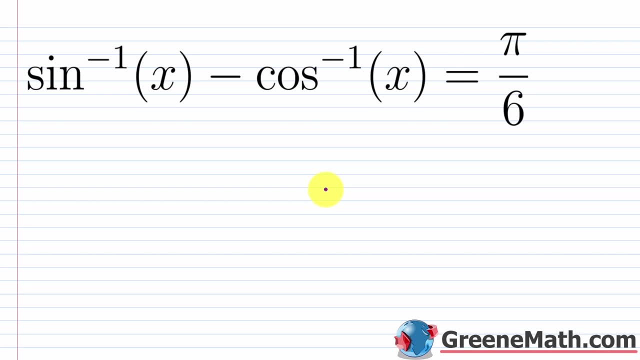 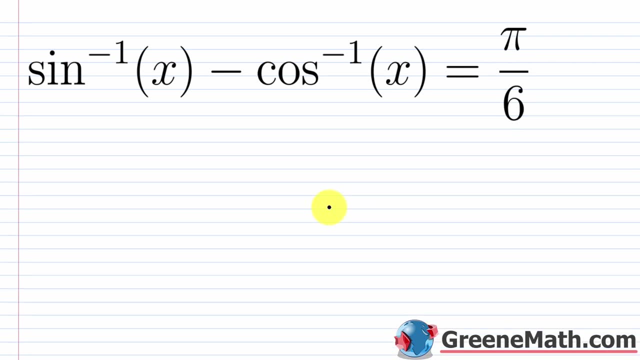 this type of problem, that you do it the long way so you can get a full understanding of what's going on And then later on, when you come across these problems again, you can just use the identities and go a lot faster. All right, so let's look at the inverse sine of x minus the inverse cosine of. 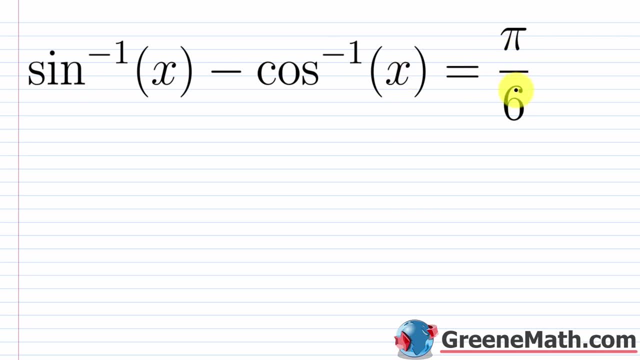 x, and this equals pi over six. So what should we do first if we get a problem like this, Pick one of these guys. So it could be the inverse sine of x or the inverse cosine of x, and you're going to isolate that on one side. So in this case, I'm going to isolate the inverse. 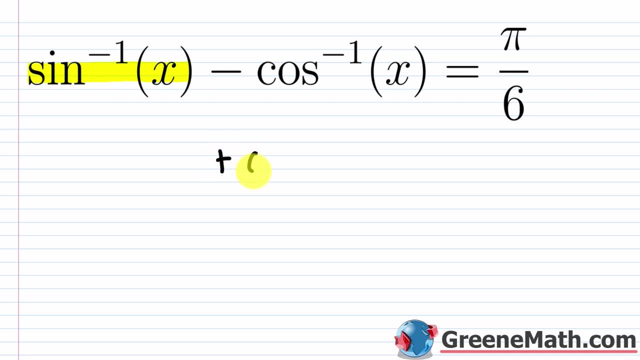 sine of x. and to do that, I'm just going to add the inverse cosine of x to both sides of this equation, So I'm going to go ahead and show this as canceling. So now I'm going to write this: as the inverse sine of x is equal to over here, I'm going to have the inverse cosine of x and then 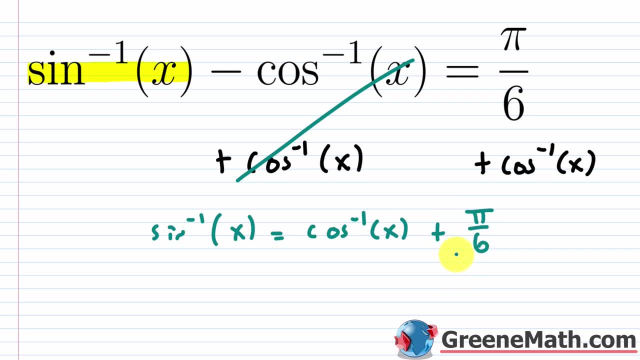 plus pi over six. Now I'm going to end up taking the sine of x and I'm going to add the inverse sine of each side. But before I do that, let me just grab this real quick and let me paste this in: I want to write this in a way to where it's crystal clear what we're doing and what everything. 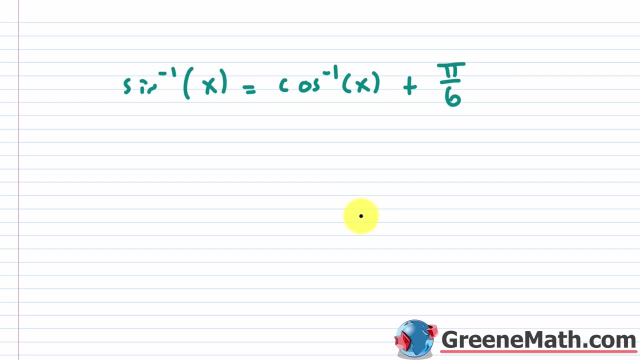 means. So I'm going to make a little substitution. You've seen me do that already. So the inverse cosine of x. we know that that's an angle from zero to pi, where zero and pi are both included, where the cosine value is x. So in other words, I can let something like theta or in this case, 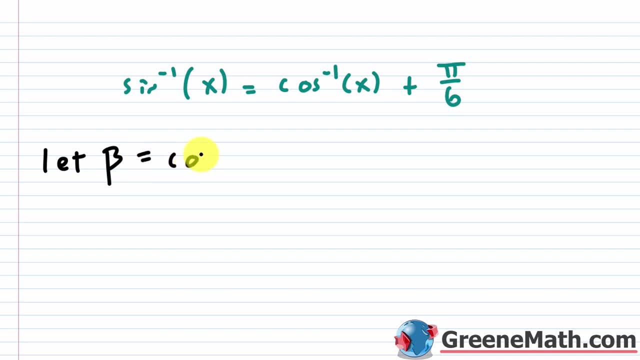 let's just use beta. So let's let beta be equal to zero, and then plus pi over six, So I'm going to equal to the inverse cosine of x. So then what I can say is that the cosine of beta is going to be. 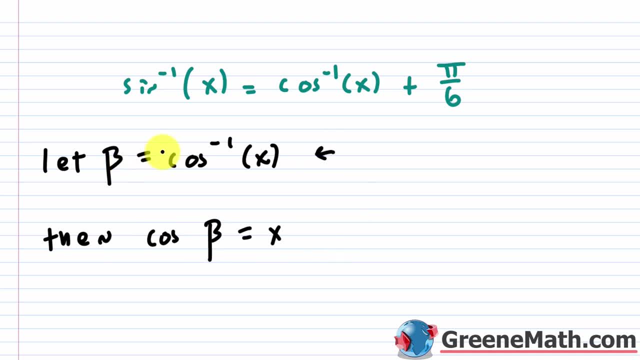 equal to x. I know that in terms of beta, right now, just looking at this, beta is going to be from zero to pi, where zero and pi are both included. That's coming from the range of the inverse cosine function. So let me say that beta is greater than or equal to zero and less than. 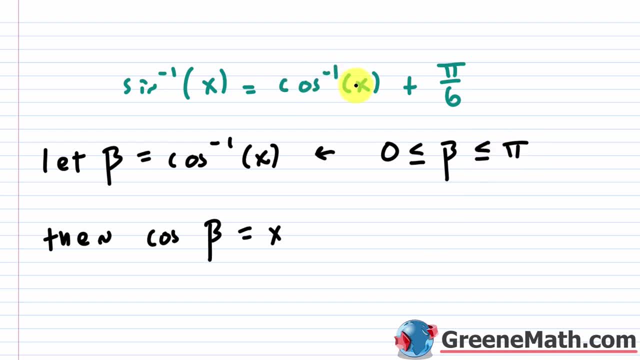 or equal to pi. So I'm just going to change this from the inverse cosine of x to the inverse cosine of x to beta. So I'm going to erase this and just put this right now as beta. Okay, let's put this over here like this. Now there's something else that you have to consider. Let me actually grab. 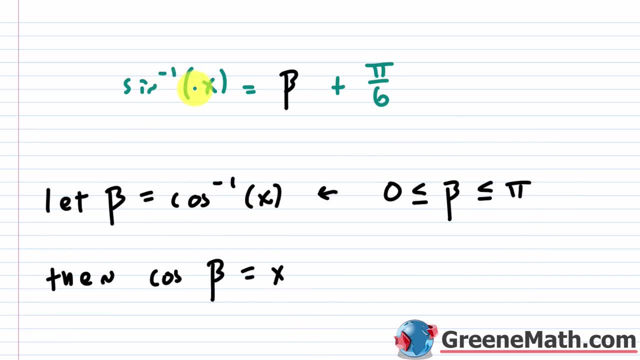 this and slide it down right here. If I have the inverse sine of x, that's going to give me something from negative pi over two to pi over two where both of those guys are included. So that tells me that this right here, this beta plus pi over six, has to be greater than or equal to. 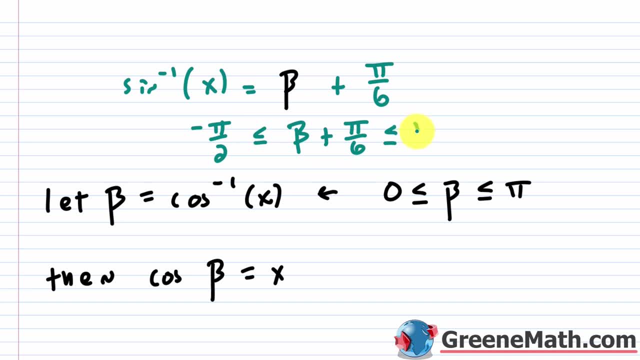 negative pi over two and less than or equal to pi over two. I'm going to put this in terms of beta being in the middle of that guy. So to do that, I'm just going to subtract pi over six away from each part of this guy Over here. let me just add negative pi over six. that would be the same. 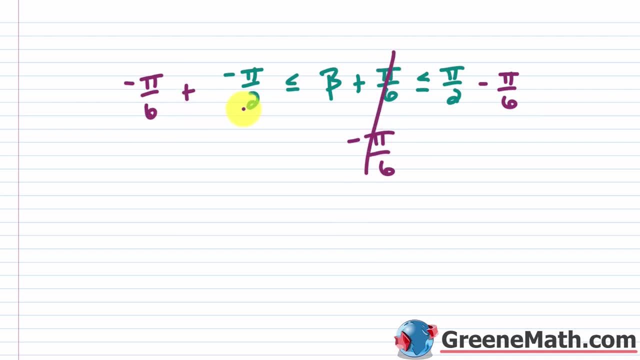 thing. So basically this would cancel, And over here I'd want to get a common denominator. So multiply this by three over three, And over here I'd multiply this by three over three as well. So I would end up with negative pi plus negative three pi over the common denominator of. 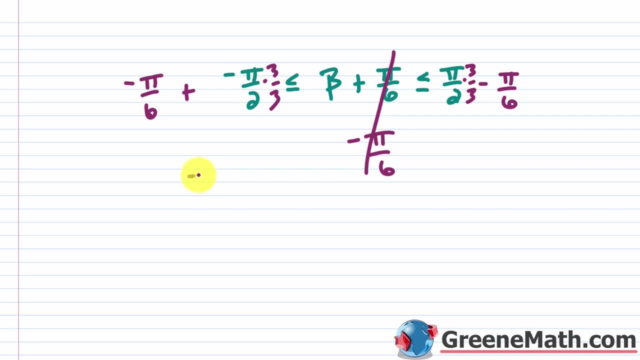 six. So that's negative. four pi over six. So this would be negative. four pi over six. And of course each guy here is divisible by two. So four divided by two is two. So this would be negative. two pi over six divided by two is three. So let me erase all of this and put this as negative. two pi over 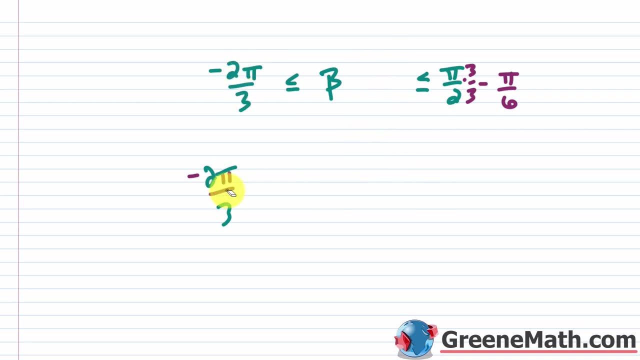 three, And let me erase this. And over here let's think about what we have. So this would be three pi minus pi over the common denominator of six. So this would be two pi over six, So two pi over six. each is divisible by two. 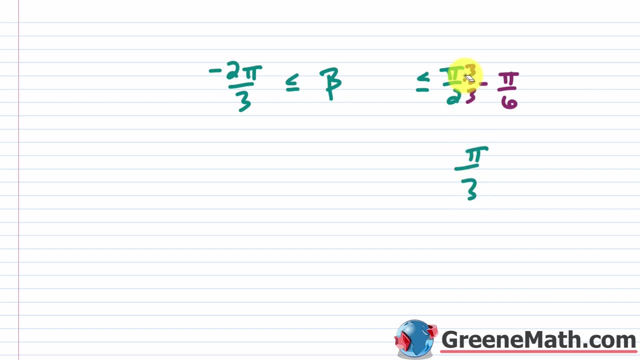 So two divided by two is one. six divided by two is three. So this is pi over three. So this is pi over three. Let me actually write this up here, And I'm going to write this a little bit more concisely, And let me come back up here And let me paste this in here, And I'm just going to arrow. 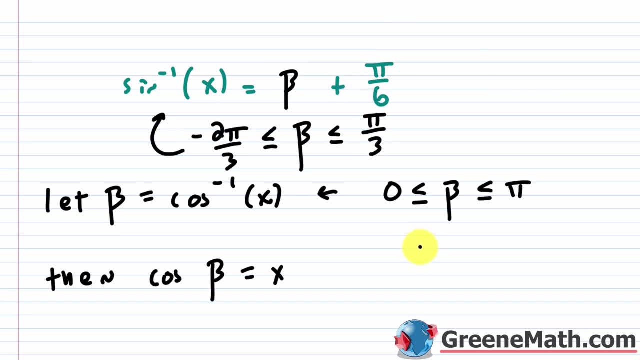 to that guy right there. Maybe this will do us some good later. All right, a little amount of one over here for our donations. First, let me write down this right here. All right, So let's make sure that we're added up And again. now. therefore, as I saw in the last, 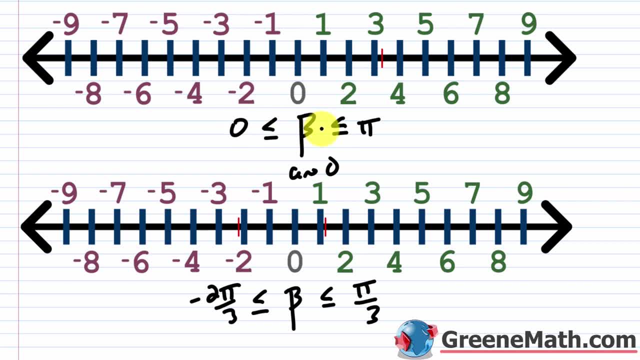 ad the inverse cosine point is greater than or equal to zero. So if vuelta was greater compared to pi over three, that would be zero over three as well. You can separate negative two off the two, So let here. So beta is greater than or equal to 0 and less than or equal to pi, So that would look like: 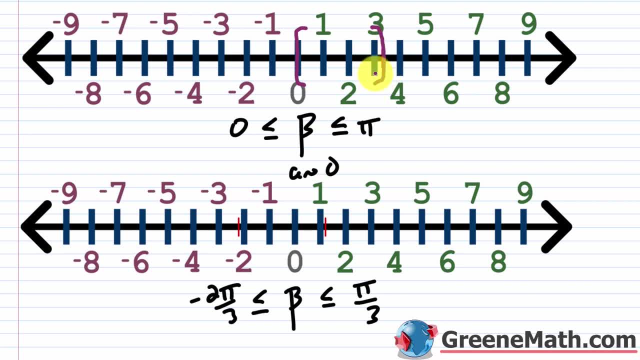 this graphically. So here's 0 and here's pi Again. that's about 3.145.. Let's just say it's about right there. So this would be about pi, right there. So this is what that looks like. if you were to graph that inequality, Then for this one beta is greater than or equal to negative. 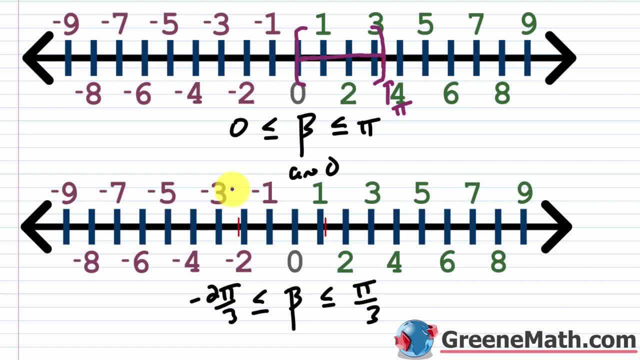 2 pi over 3 and less than or equal to pi over 3.. Let's say that this right here is about negative 2 pi over 3.. And let's say that this right here is about pi over 3.. Just in case you're curious. 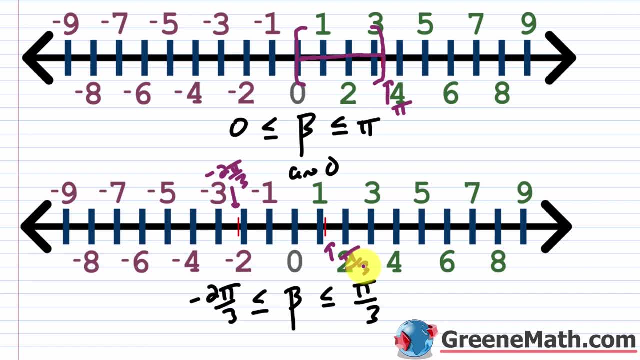 negative 2. pi over 3 is about negative 2, point, let's say 0.9.. And pi over 3, that's about, let's say, 1.05.. So graphically this would look like this right here, So this right here. 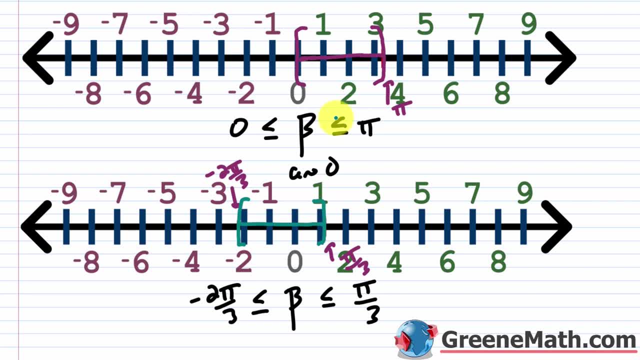 if you want to look at that, inequality so something like that. So if I want the intersection of the two, again, I'm looking for values that are going to work in between. In other words, it would have to satisfy this one and this one. So when I set that up, 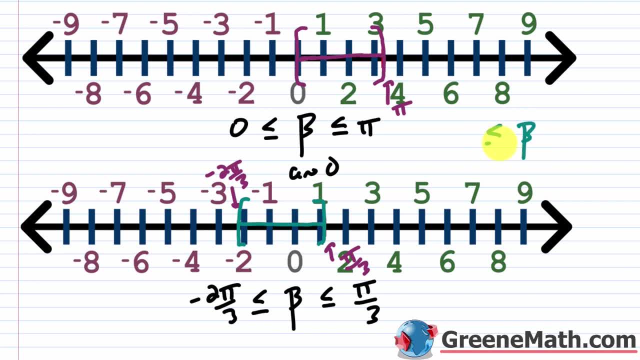 I'm running out of room, but let me just do it. over here. I would say that beta is greater than or equal to what. Well, consider that over here you have a 0 and over here you have a negative 2 pi over 3.. Well, it's got to be 0. It's got to be the one that's more restrictive or further to. 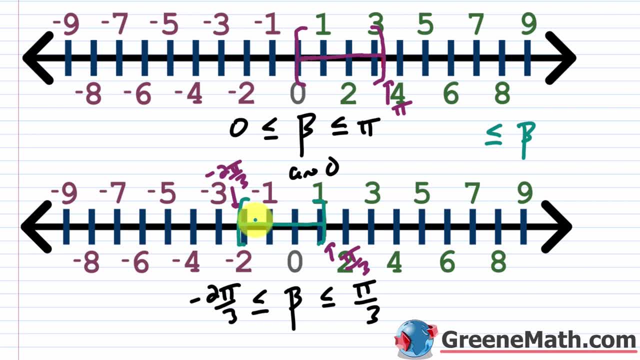 the right, because it's got to work in both. If I had a value that was, let's say here, that was to the left of 0, but to the right of negative 2 pi over 3,, well, it would work in this one. 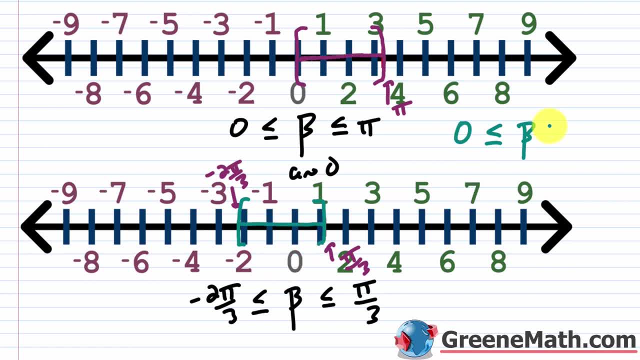 but it wouldn't work in this one, So I'm going to have to choose 0 here and then I say it's less than or equal to well for this one. I want the one that's further to the left right, because it's going to be more restrictive and include fewer values. 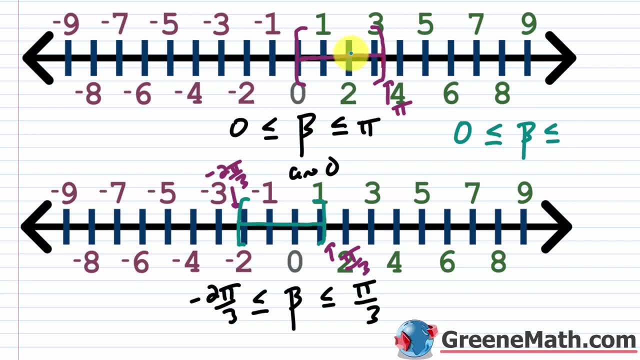 So I want the pi over 3.. In other words, if I had something like, let's say, 2, that was to the right, of pi over 3, well, it works in this one, but doesn't work in this one, So it's got to work. 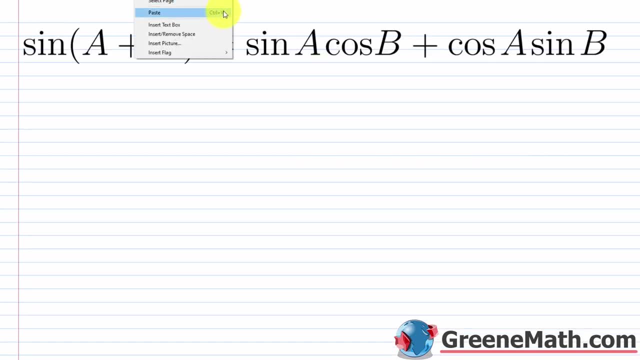 in both. So I'm going to choose pi over 3.. Okay, let me come down here and I'm going to paste this in and I'm coming back to this in a second, and let me grab this and let me come down here. 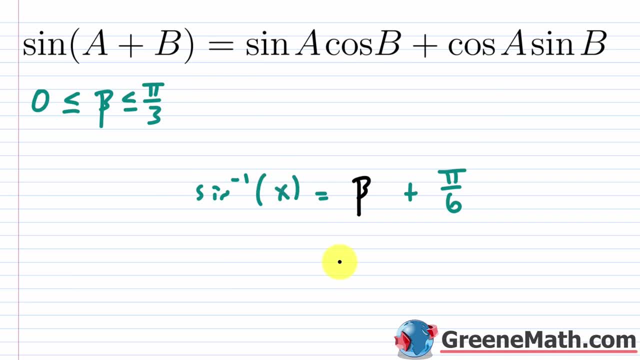 and paste this in. So we're going to need this identity. That's why we're going to need this identity. So I have that set up already. So what I'm going to do now is take the sine of each side. So I'm going to take the sine of the inverse sine of x, and this is equal to the sine of beta plus. 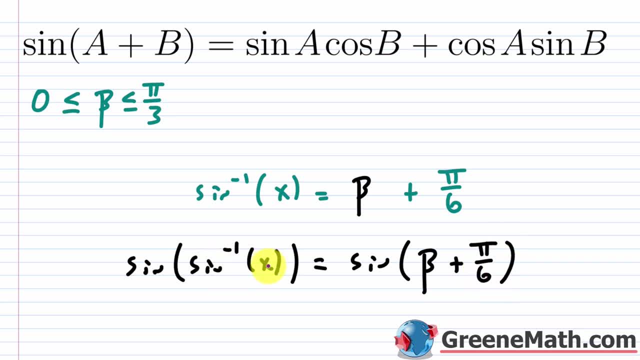 pi over 6.. When I think about this guy right here again from the cancellation property that we talked about earlier, this will undo this as long as x is in the domain of the inverse sine function. So from negative 1 to positive 1, with both being included. So let's go ahead and say: 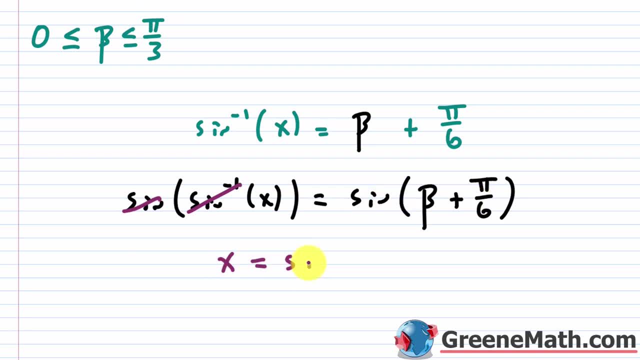 that x is equal to this guy right here, So the sine of beta plus pi over 6.. Now I'm going to erase this, and now we're going to use this sum identity for sine to simplify this. So what I'll do is say: 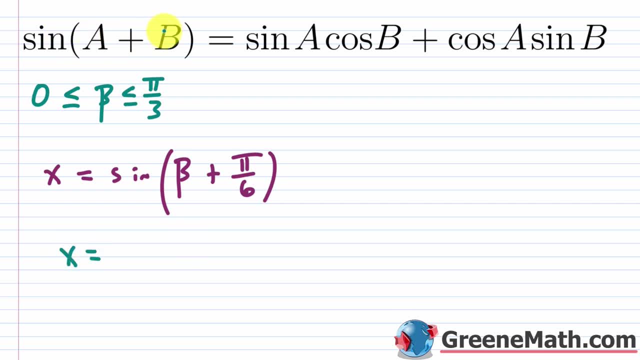 that this is x is equal to. again, if you have the sine of a plus b, it's equal to the sine of a times the cosine of b plus the cosine of a times the sine of b. So this would be the sine of the. 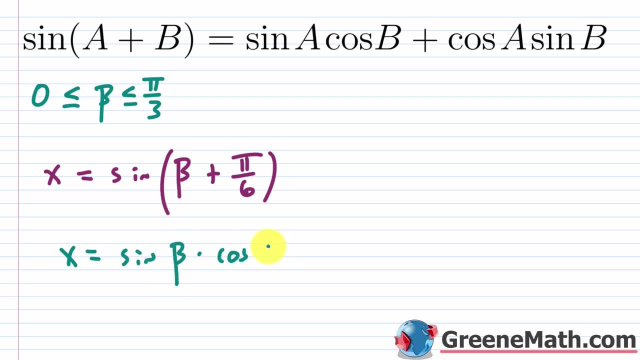 first guy, which is beta, and then times the cosine of a, times the cosine of b, So that's the cosine of the second guy, which is pi over 6, and then plus the cosine of the first guy, which is beta, and then times the sine of the second guy, which is pi over 6.. Now I know most. 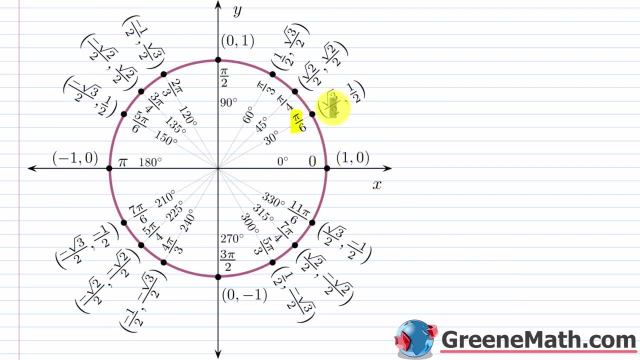 of you know this. but if you go to pi over 6 on the unit circle, the x-coordinate is the cosine value, so that's square root of 3 over 2, and the y-coordinate is the sine value, so that's 1 half. 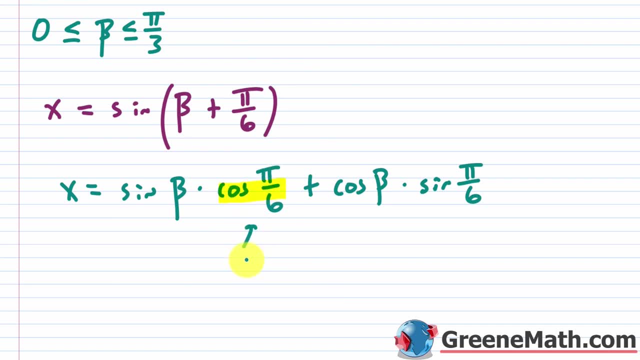 So, coming back up here, I can replace the cosine of pi over 6 with square root of 3 over 2, and I can replace the sine of pi over 6 with square root of 3 over 2, and I can replace the. 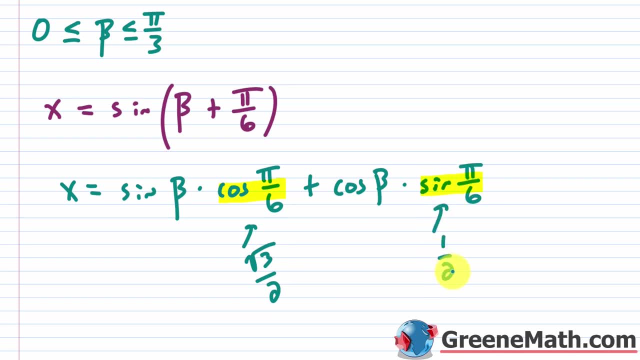 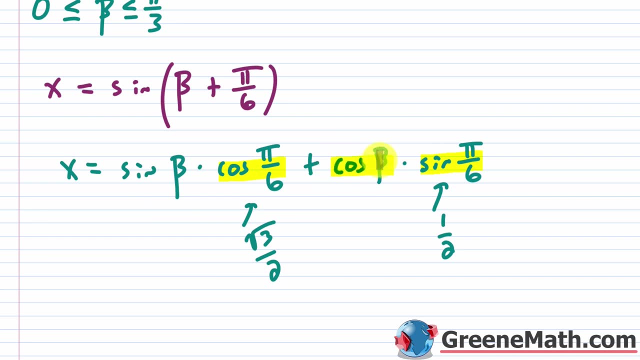 sine of pi over 6 with 1 half. So this right here is 1 half. Now we also know what the cosine of beta is. so the cosine of beta again is going to be x. So this right here is going to be x. 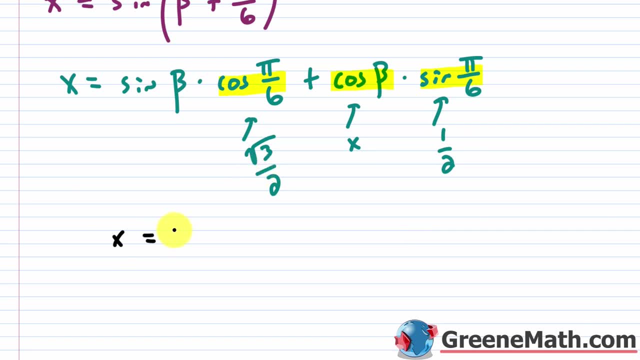 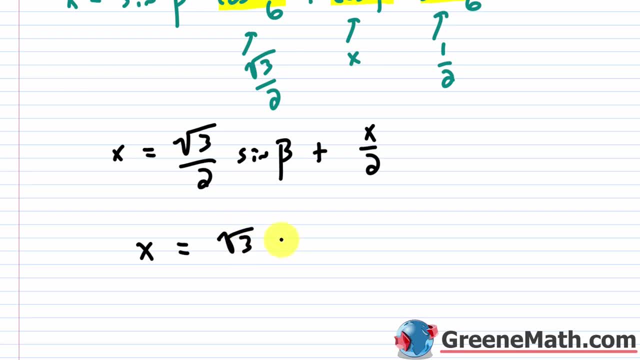 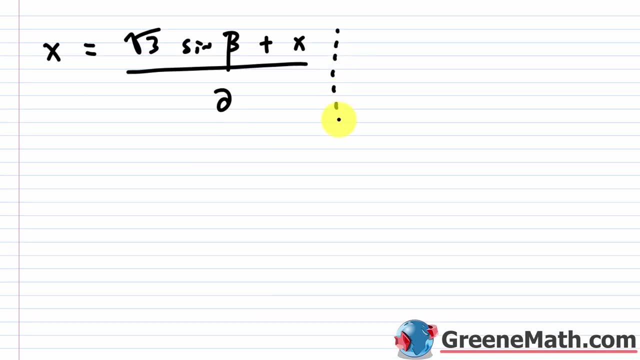 say, x is equal to the square root of 3 times the sine of beta, plus x over the common denominator of 2.. So the question now is: what is the sine of beta? So that's the holdup. So what is the sine? 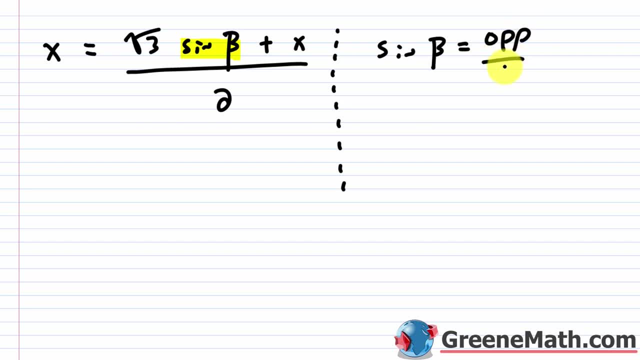 of beta. So again, this is the opposite. over the hypotenuse. Do we know what the hypotenuse is? Remember the cosine of beta. the cosine of beta is equal to your x over 1, right, Because x can be written as x over 1.. And this right here is your adjacent, And this right here is your. 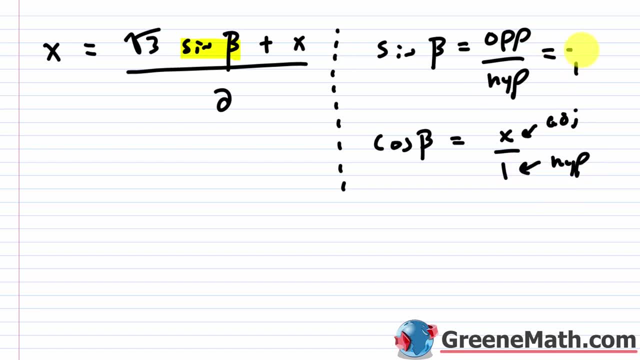 hypotenuse. So I know the hypotenuse is 1.. So let me put that there. Now, what about the opposite? Can I figure that out? Remember that we said that beta is greater than or equal to 0 and less than. 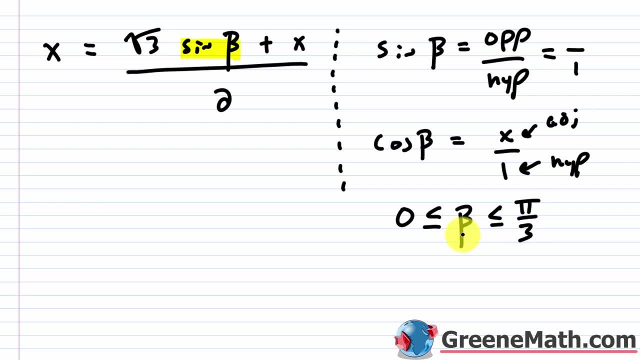 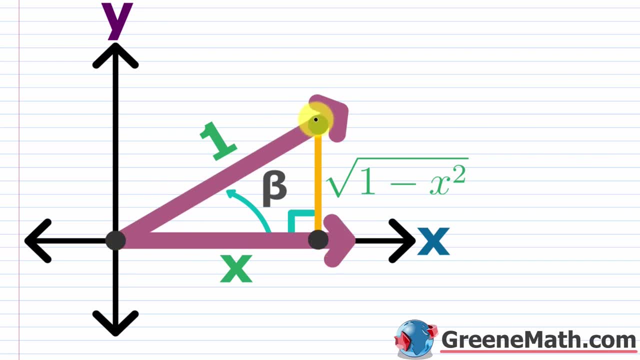 or equal to pi over 3.. So I'm just going to sketch a triangle in quadrant 1. And it would look something like this: So your adjacent is just going to be x, Your hypotenuse is going to be 1.. And you're going to find through the Pythagorean theorem, 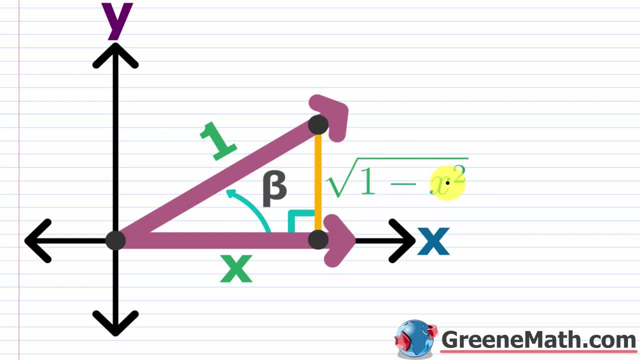 that the opposite is going to be the square root of 1 minus x squared. So again, if you want to go through this, let's say that we label this right now generically as y, So we would say that we have x squared. So I'm just calling this length right here x, So it's x squared Plus. 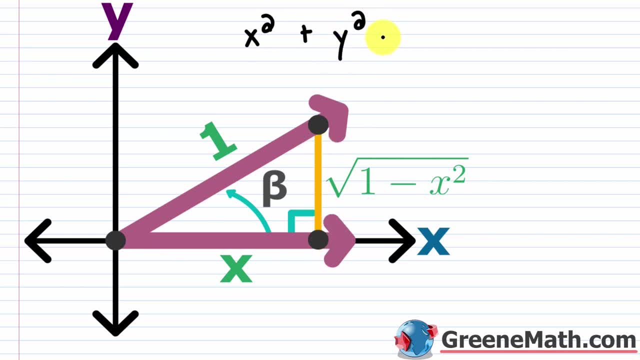 I'm going to have this guy right here. Let's call that y. So y squared is equal to this guy right here. your hypotenuse: We know that's 1. So 1 squared. You're going to solve this for y. So you're just going to subtract x squared away from each side of the equation. 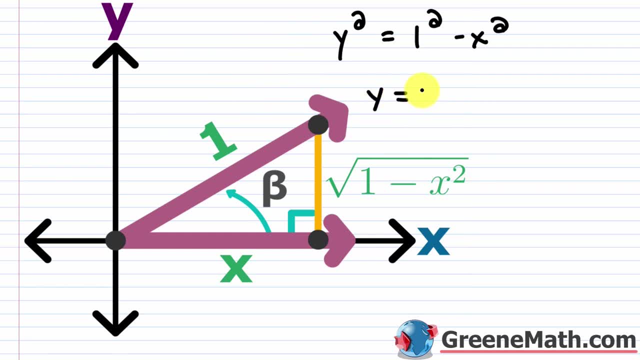 I'm just going to erase this And then to solve for y. you want the principal square root of this guy right here. So 1 squared is just 1 minus x squared, And the reason for that is again: your y value is never going to be negative because beta is greater than or equal to 0. 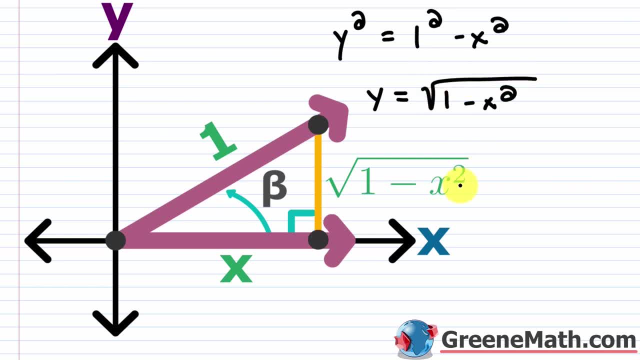 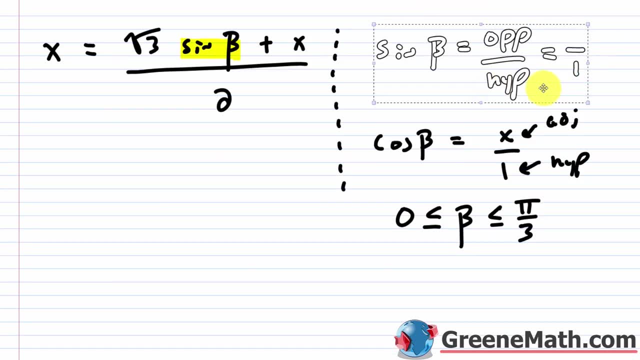 and less than or equal to pi over 3.. So you use the principal square root here. So this right here gets for your opposite: the square root of 1 minus x, squared. Let me actually move this over. I don't think it'll fit. I'm just going to say that this is the square root of 1 minus x squared. Let me. 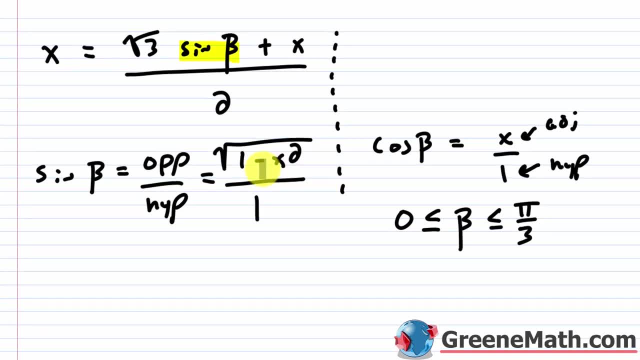 make this a little bit longer here. So this is over 1.. So what I would do now is plug this right here in for that sine of beta, And then we would just solve for x. What I want to do is say that x is equal to the square root of 3. And then times again for the sine of beta. 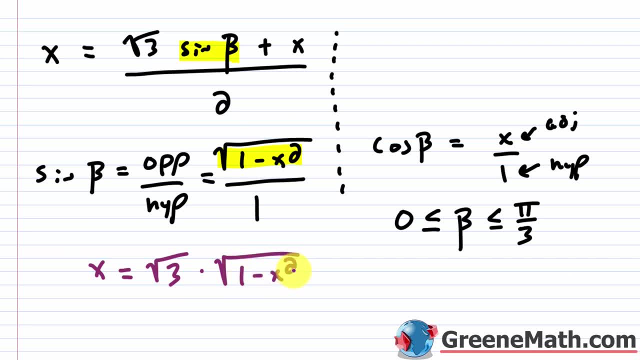 I have the square root of 1 minus x squared. If you want, you can combine those now. I think it'll make it a little bit easier to understand. Again, if you have the square root of a times the square root of b, we know this is the square root of a- b, So the square root of 3 times the square. 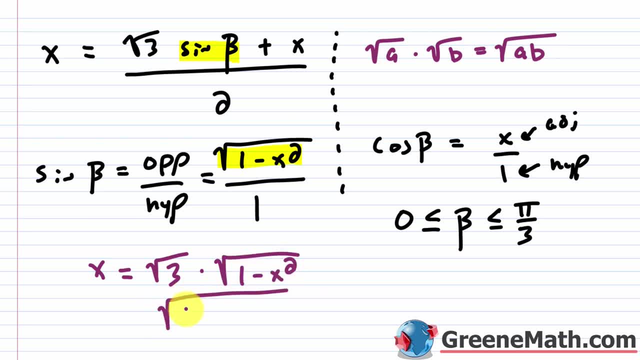 root of 1 minus x squared would be the square root of 3 times the quantity 1 minus x squared. And if you distribute that 3 into each guy, you would have the square root of 3 minus 3x squared. So again, 3 times 1 is 3.. And then minus 3 times x squared that's 3x squared. 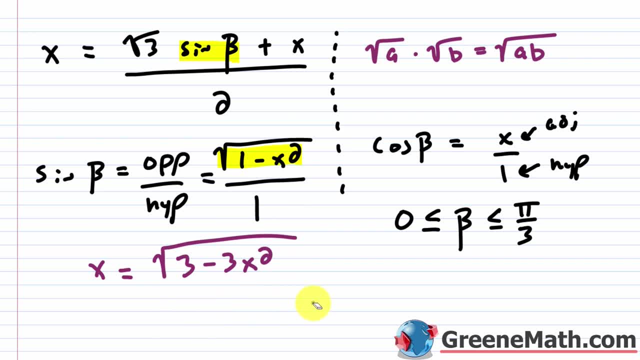 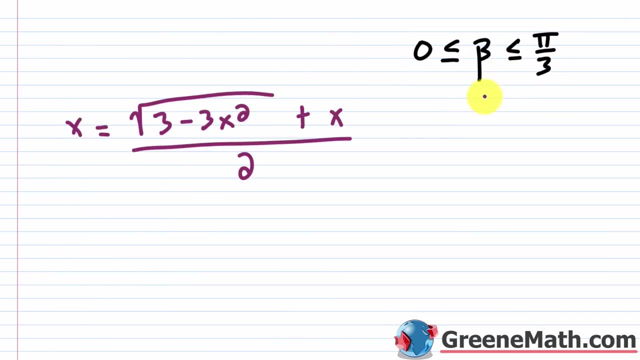 Let me make this a little bit better here And let me erase this and also erase this. So then we would say: plus, you have this x here, And then this is over 2.. Now I want to grab this guy right here And let me come down to this sheet here. The reason I'm keeping this here is because we're 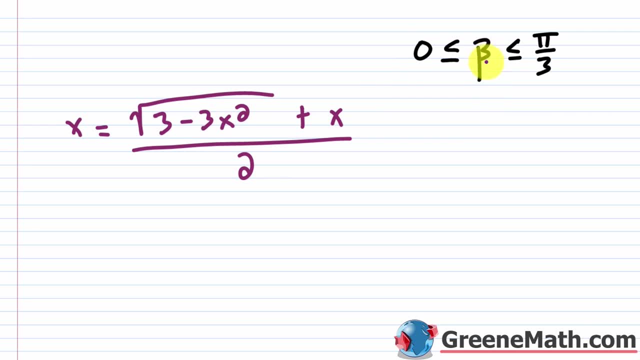 going to end up squaring both sides of our equation And we want to remember that our angle beta, which represents the angle of the square root of b, is equal to the square root of b. So inverse cosine of x that is greater than or equal to 0 and less than or equal to pi over 3.. 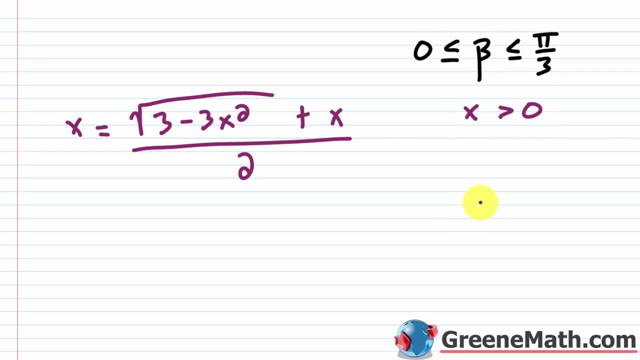 So I know that my x values here are greater than 0. So just keep that in mind. So for this one right here, I'm going to multiply both sides by 2.. Let me put a little border and section this off. So multiply over here by 2. And of course this is going to cancel away. And so now we'd say that: 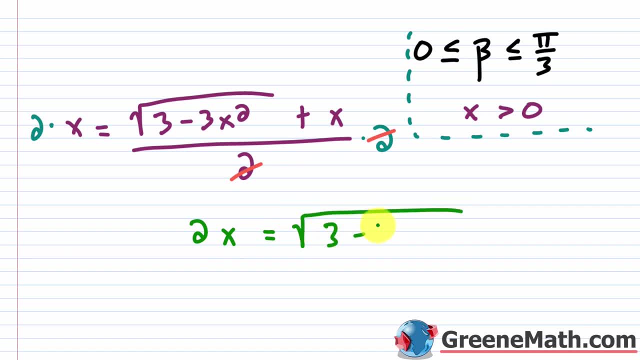 we have: 2x is equal to the square root of 3 minus 3x squared, and then plus x. At this point I would subtract x away from each side of the equation, And so this right here is going to cancel. So 2x minus x is x, So x is equal to the square root. 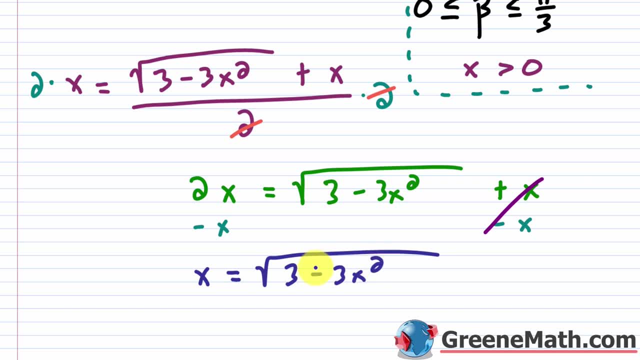 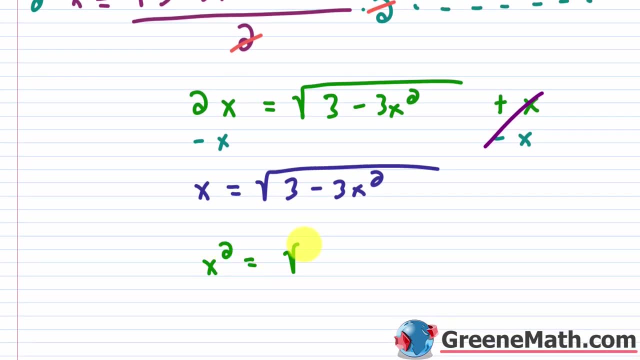 of 3 minus 3x squared. Now I want to square both sides. So what that would give me- let me come down here a little bit- is: x squared is equal to the square root of 3 minus 3x squared. 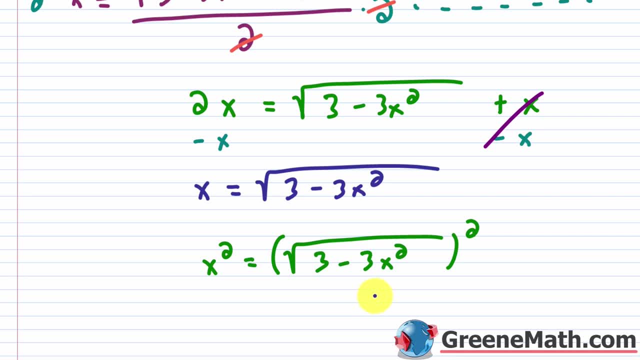 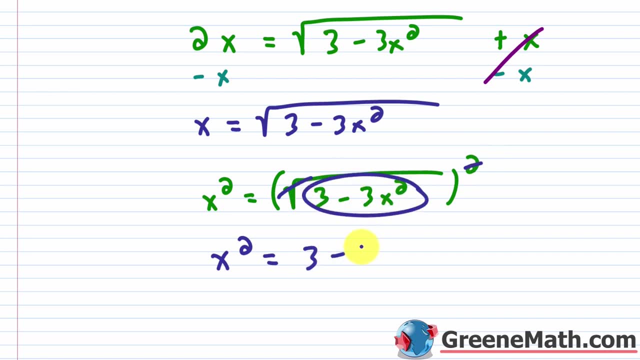 And again I'm squaring this as well. So just squaring both sides of our equation And that's going to give me x squared is equal to. So you're left with that radicand there. So 3 minus 3x squared. Let me make this 3 a little bit better there. So at this point, 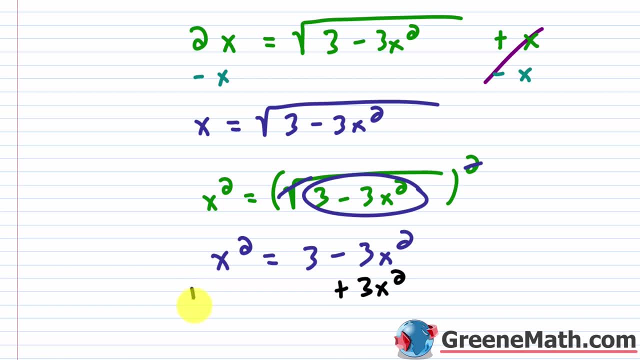 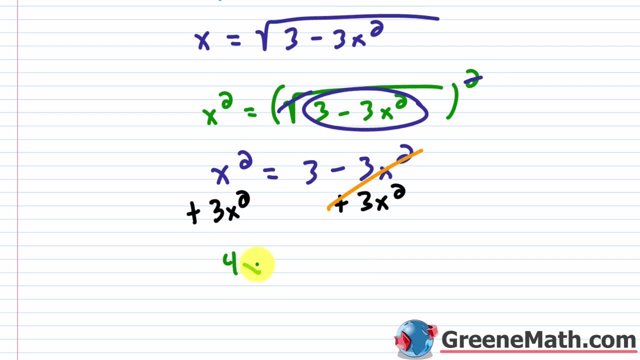 I just want to add 3x squared to both sides of the equation. This is going to cancel, And so you have x squared plus 3x squared. That's going to give me 4x squared, And this equals over here. I just 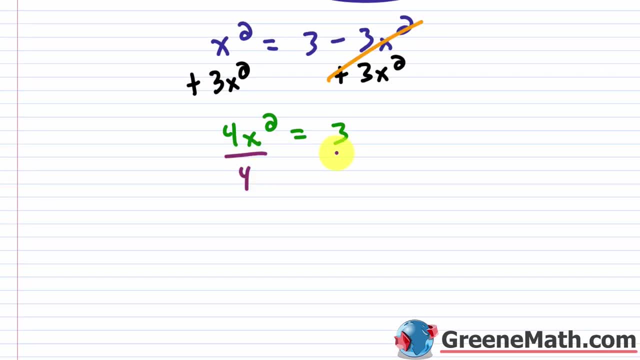 have 3.. Now, if you want to solve for x, you divide both sides of the equation by 4. This would cancel. You're going to get x: squared is equal to 3 fourths. Now here's where we need to. 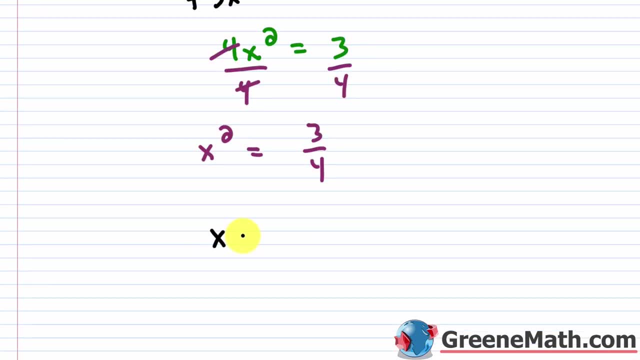 think, Remember, with the square root property we would say that x is equal to plus or minus the square root of 3 fourths. So this turns into plus or minus the square root of 3.. So the square root of 3 over 2.. Do I need the plus or minus here? No, Because again I cut it off. But we said: 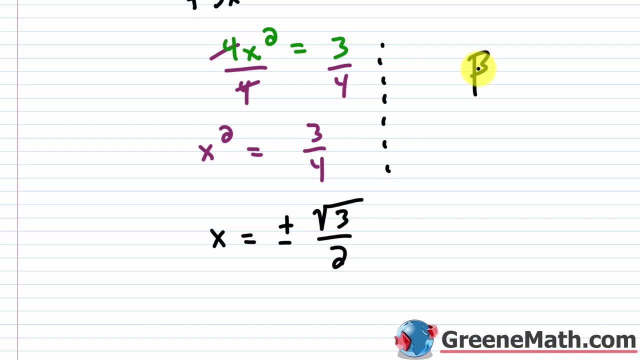 that beta, which was our inverse cosine of x, is greater than or equal to 0 and less than or equal to pi over 3, which told me that x is going to be greater than or equal to 0.. So I'm going to. 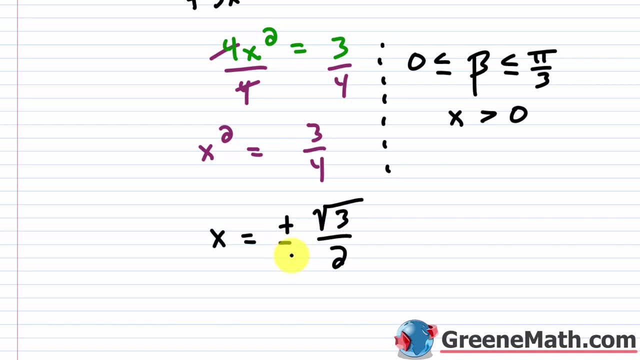 be greater than 0.. So what this tells me is that I don't need the negative of the square root of 3 over 2.. That guy is not going to work. It's going to be an extraneous solution. It's something that 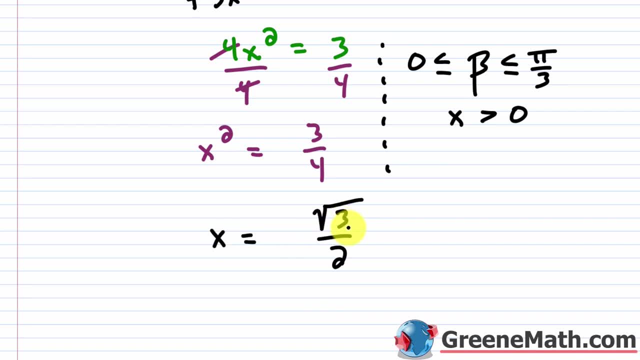 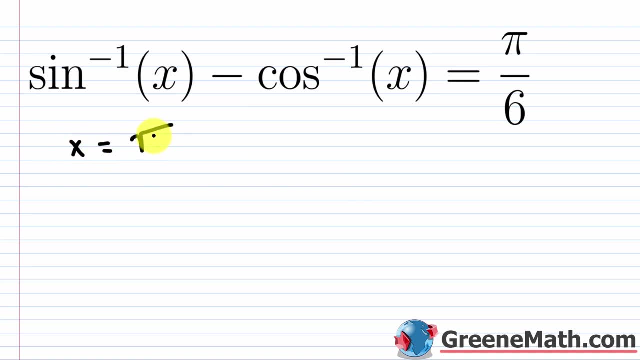 was produced because we squared both sides of our equation. So you just get: x equals the square root of 3 over 2.. All right, So for these problems again, I always recommend you check them. So let's put: x is equal to the square root of 3 over 2.. Let's just make sure that it works Again. 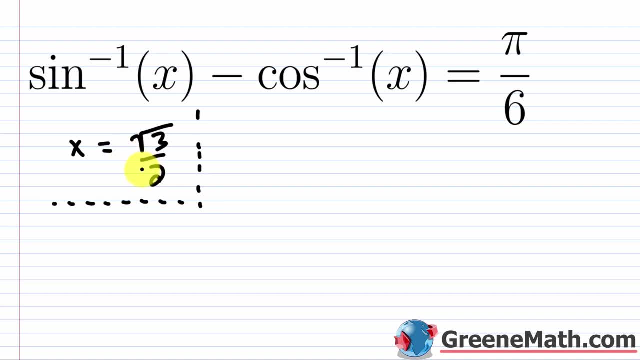 if you were to try to check, x equals the negative of the square root of 3 over 2, the extraneous solution there. it's not going to work. Remember that x values. it would be positive when we're dealing with this angle beta. So what I would think about here is: 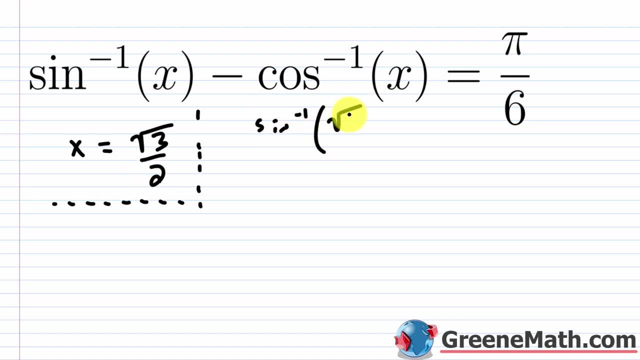 what is the inverse sine of this square root of 3 over 2?? A lot of you know that it's going to be pi over 3.. We'll go to the unit circle and grab it, And then what is the inverse cosine of square? 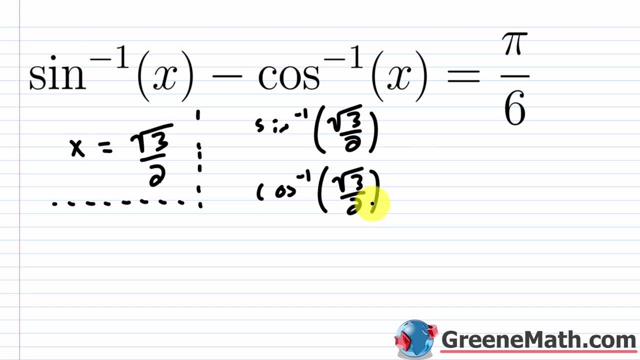 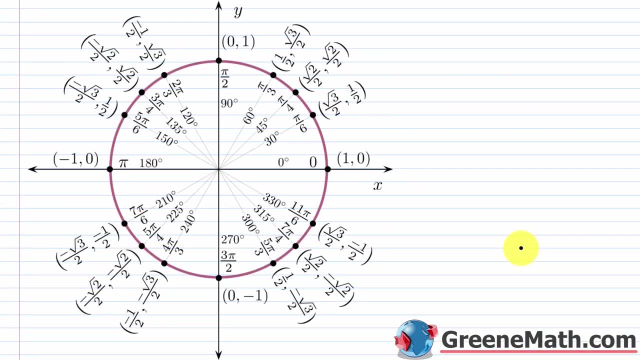 root of 3 over 2? Most of you know that's pi over 6.. So let's put this as pi over 3.. Let's put this as pi over 6.. Let's go to the unit circle real quick, just in case you need it. So again for. 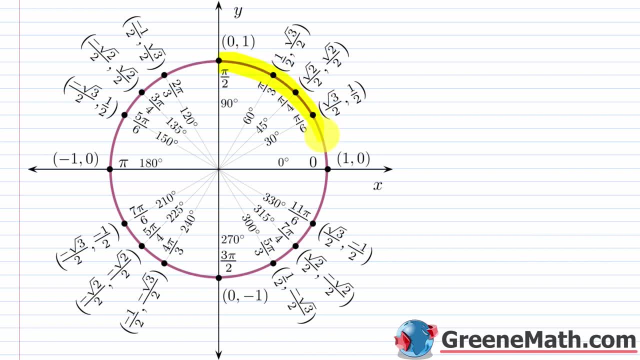 sine of square root of 3 over 2, I'm working from negative pi over 2 to pi over 2.. And I'm looking for a sine value of square root of 3 over 2.. So that's going to be right here, right here, And the 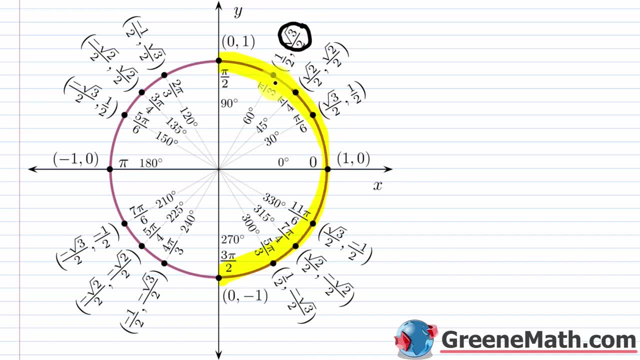 associated angle, again in this interval from negative pi over 2 to pi over 2, is going to be pi over 3.. So that tells me that the inverse sine of the square root of 3 over 2, again is pi over 3.. And then for the inverse cosine of the square root of 3 over 2, again with 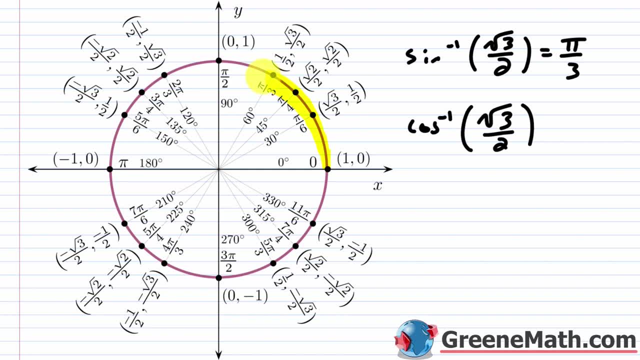 this one. now I'm working from 0 to pi. Both of those are included, So from 0 to pi. And again, where do I have a cosine value of square root of 3 over 2?? Well, that's going to be right here. 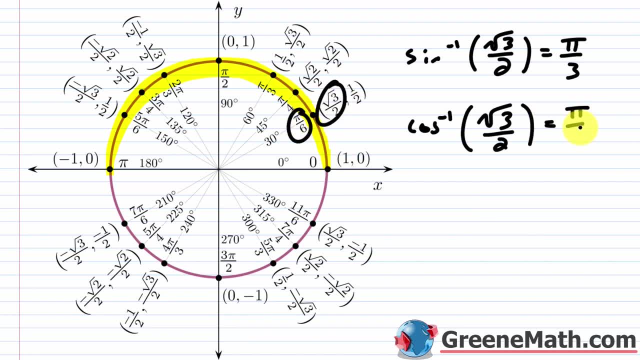 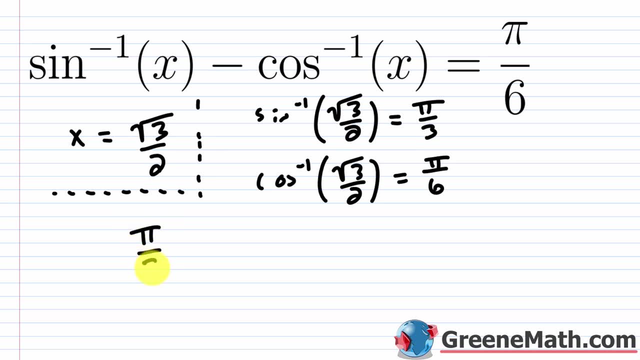 at pi over 6. So this would end up being pi over 6.. All right, so now let's just plug in. So the inverse sine of square root of 3 over 2 is pi over 3.. So that is pi over 3.. And then you'd have. 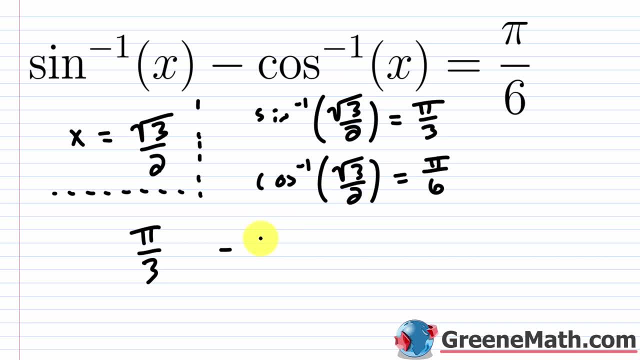 minus the inverse cosine of square root of 3 over 2. That's pi over 6.. Does this equal pi over 6?? Well, if I get a common denominator here, I'd multiply this by 2 over 2. And so that. 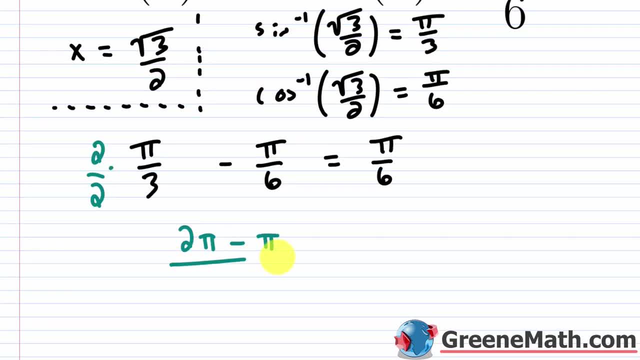 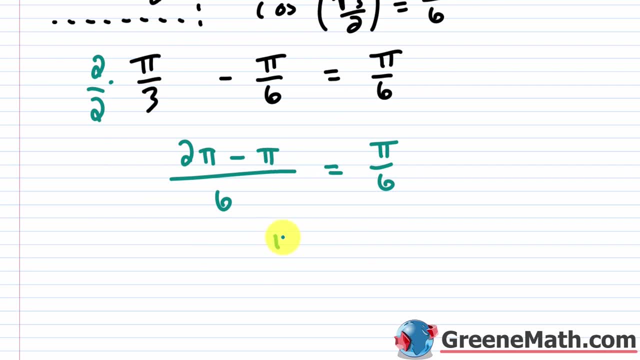 would give me 2 pi minus pi over the common denominator of 6.. Does that equal pi over 6?? Yeah, 2 pi minus pi is pi. So this would be pi over 6 is equal to pi over 6,, which is a true. 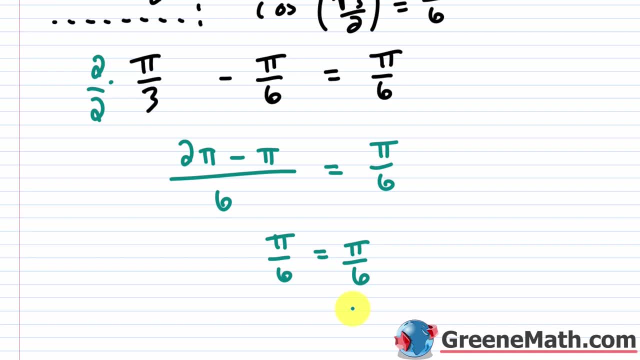 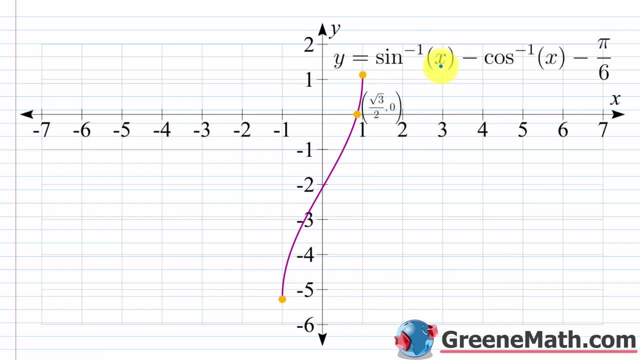 statement. So that solution x equals square root of 3 over 2 is a valid solution. Again, you can always verify this graphically. So you can set this up as: y equals the inverse sine of x minus the inverse cosine of x minus pi over 6.. Where did that come from? 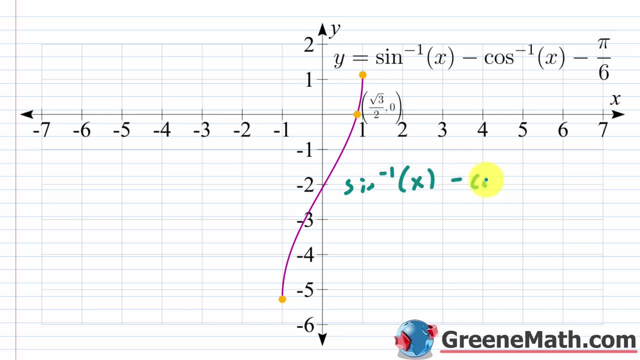 Again, if you have your inverse sine of x minus, your inverse cosine of x is equal to pi over 6.. Well, if you subtract pi over 6 away from each side of the equation, this would become: minus pi over 6 is equal to 0.. So all I'm really doing here is plugging in a 0 for y, And I'm 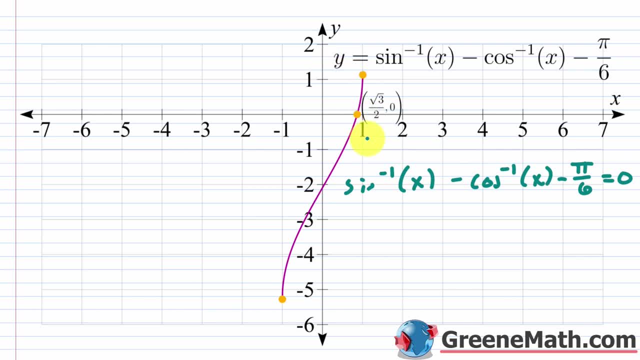 asking for which x value. am I going to get a y value of 0?? So again, that's going to be your x value. that occurs at square root of 3 over 2 comma 0. So that tells me the x value is square. 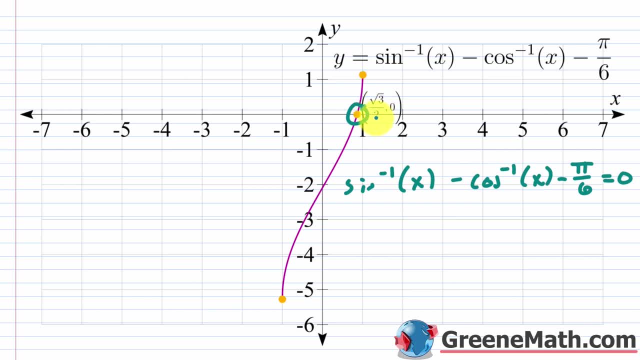 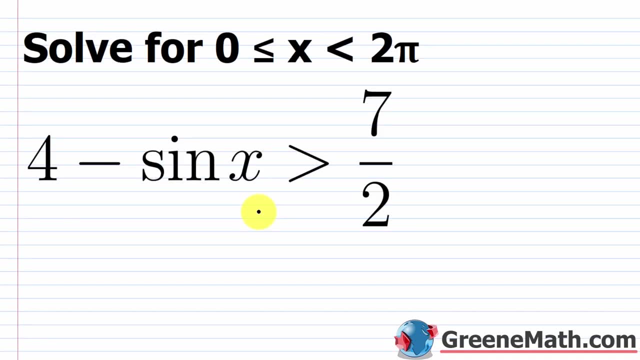 root of 3 over 2.. So this confirms my solution that x equals square root of 3 over 2.. In this lesson we want to talk about solving trigonometric inequalities. All right, let's go ahead and look at the first problem. So this will be a really simple example, just to get started. So we want 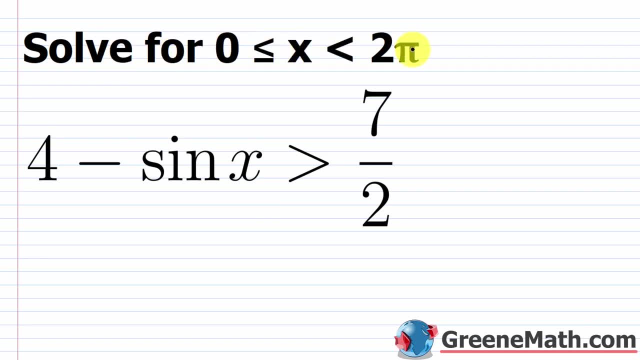 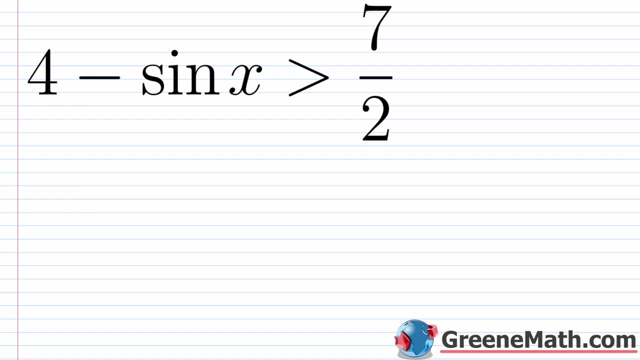 to solve for x is greater than or equal to 0 and less than 2 pi, And so we have 4 minus the sine of x is greater than 7 halves. So how do we solve something like this In this particular case? it's a very simple example, So you could isolate the sine of x on: 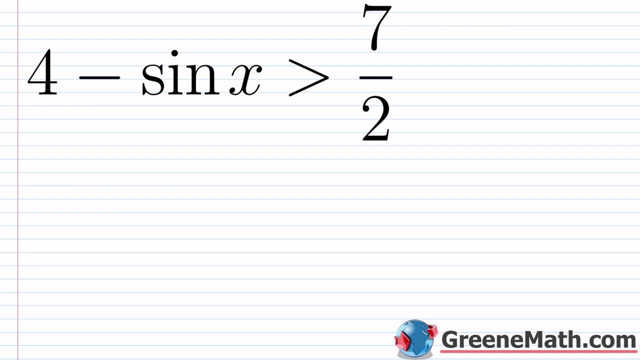 one side and then have a number on the other, And then you can go to the unit circle and get your solution that way. I'm not going to actually do that because I want to build up the concept that we're going to use for the harder examples. So what I'm going to actually do is make the right. 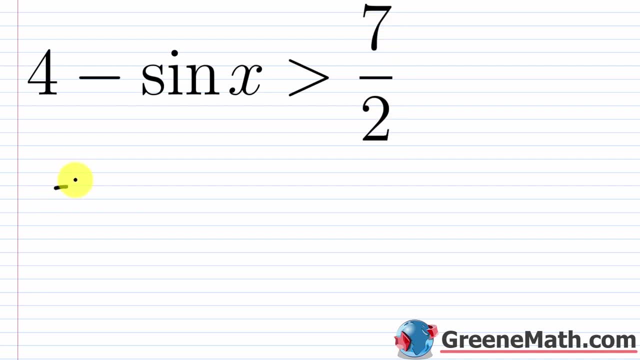 side 0 to start. So I'm going to say that I have- let's just reorder this- the negative of the sine of x and then plus 4.. I'm just going to leave a space here and put: this is greater than 7 halves. 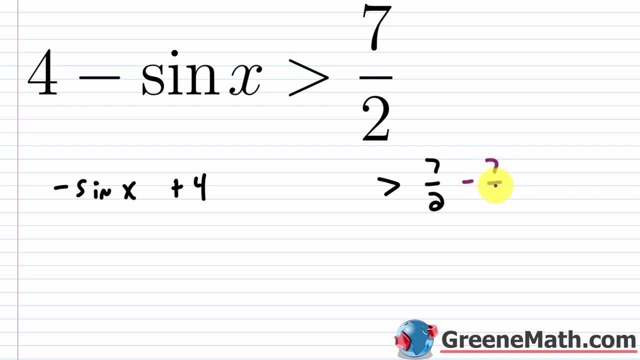 I want the right side to be 0. I just need to subtract 7 halves away from each side of the inequality. I would want a common denominator, So let me multiply 4 over 1 times 2 over 2.. Let me. 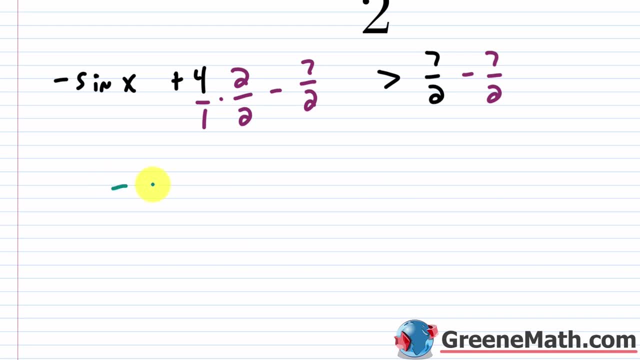 put this minus sign down here. So at this point I'm going to write that I have the negative of the sine of x And then basically, this 4 times 2 is 8.. So this would be 8 over this 2.. So 8 over. 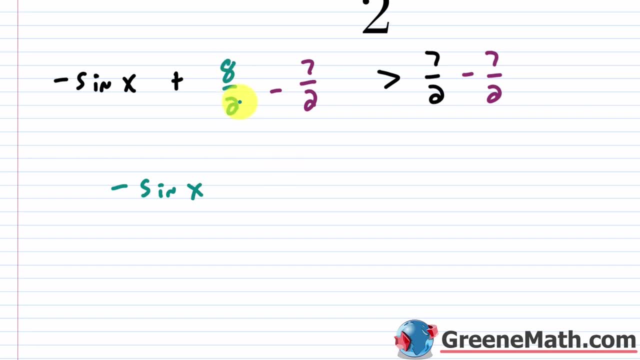 2, that's the same thing as 4.. We're just getting a common denominator And 8 over 2 minus 7 over 2, we do 8 minus 7, which is 1 over the common denominator of 2.. So that's just 1 half. So this: 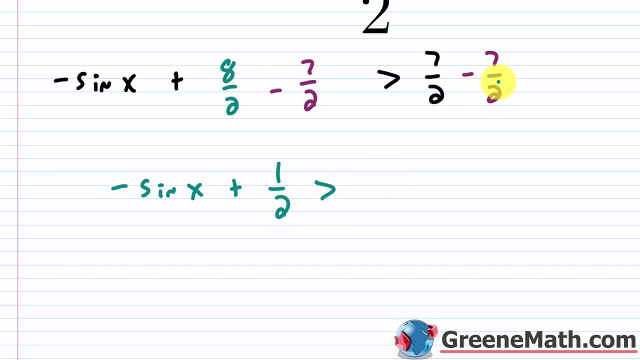 is plus 1 half, And then this is greater than 7 halves. minus 7 halves is obviously 0.. At this point, what I would do is get rid of this negative that's in front of the sine of x. I'm actually. 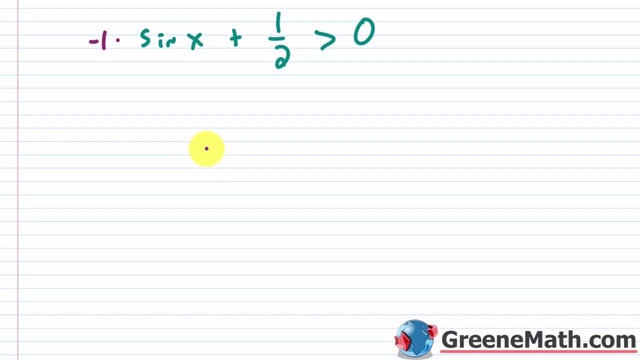 going to write this as negative 1 times the sine of x. So it's crystal clear what we're doing. I'm just going to multiply both sides of the inequality by negative 1.. Remember if you do that, you have to flip the direction of the inequality symbol. So let me write negative 1 times this negative 1. 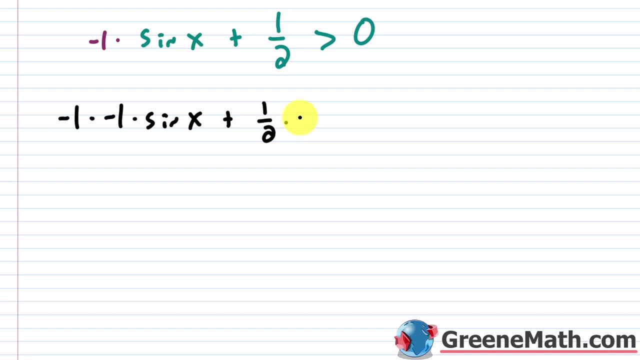 and then plus, you're going to have your 1 half times negative 1.. This is going to get flipped, So right now it's a greater than, Because we're multiplying both sides by a negative, it's going to become a less than And then you have 0 times negative 1.. So negative 1 times. 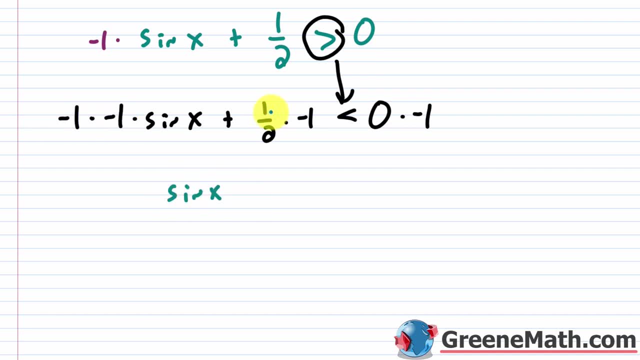 negative 1 is positive 1.. So this is just the sine of x now, And then you have 1 half times negative 1.. That's negative 1 half, And then this is less than 0 times anything is 0. So I'm going to grab. 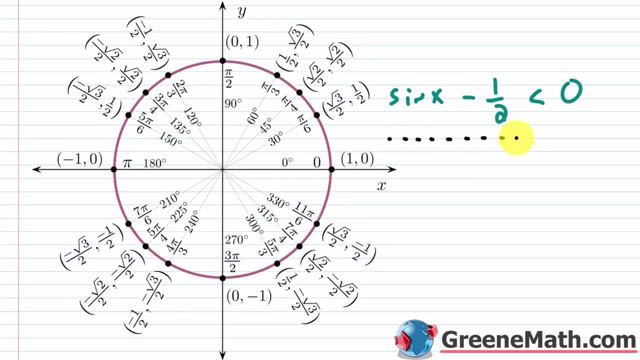 this real quick, Okay. so at this point I'm just going to come to the unit circle and put a little. Now, this is an easier example, So of course you could just figure out. well, where's the sine of x? 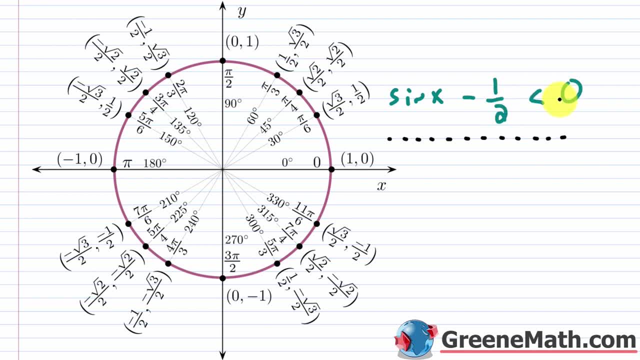 less than 1 half just by adding 1 half to both sides. I'm not going to do that Because, again, I want to build up the method that we're going to use with the more challenging scenarios. But once you have everything down in terms of what methods to use, when you can go ahead and solve. 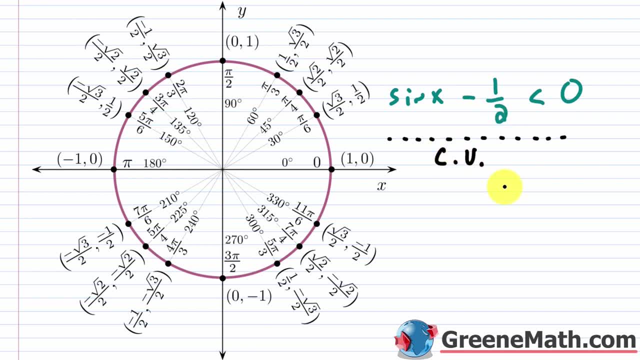 it that way, It's no problem. So I'm going to write down that we want to find the critical values here. And how do we do that? Again, you replace your inequality symbol with equals, So you would have the sine of x minus 1 half is equal to 0.. Add 1 half to both. 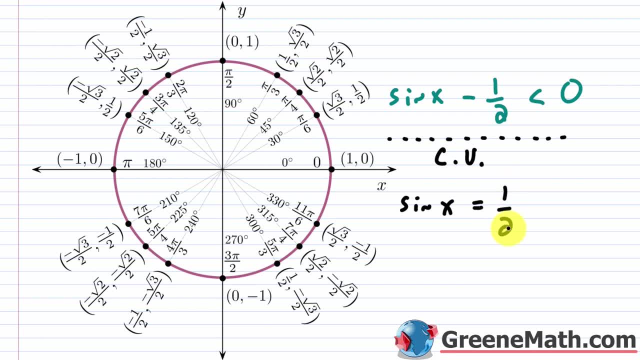 sides and you'll get. the sine of x is equal to 1 half. So basically the solutions there. if we're working in that interval, let me write that out So we know we're working from zero, and zeros included, out to two pi, and two pi is excluded. Well, your solutions there, you're. 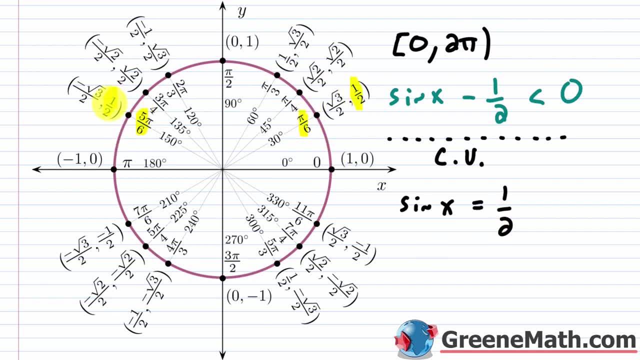 going to have pi over six, you have a sine value of a half, and then also five pi over six, you have a sine value of one half. So when I write down that the critical values are going to be where x is going to be pi over six, and then five pi over six. the reason we want to know that 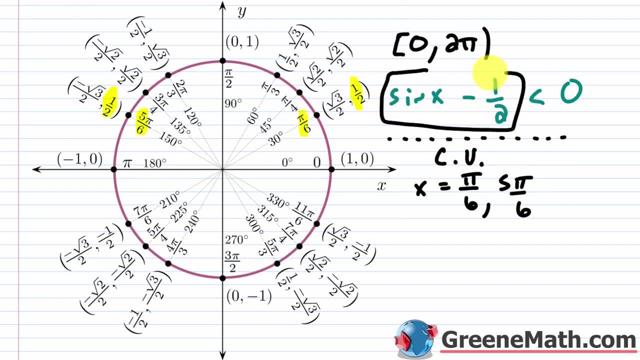 we want to know where this guy right here. the left side of this guy is going to be zero. So basically, that acts as a boundary for us And we're going to be able to set up some intervals on our number line. Or you can also do it with a table, or you can do it on the unit circle. 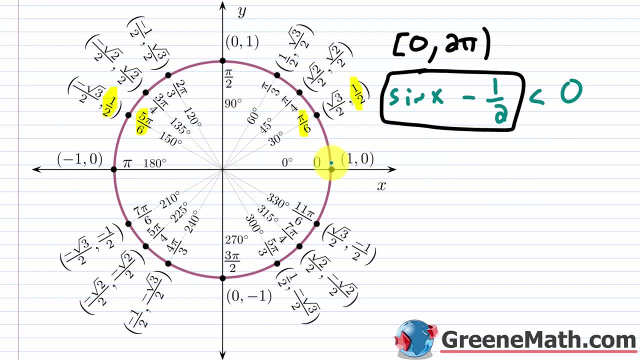 you could split this up and say: okay, well, one interval is going to be from zero to pi over six, and I'm going to exclude everything for right now. So basically you'd have an interval from zero to pi over six. So that's one of them, And then another interval you would take from pi over six. 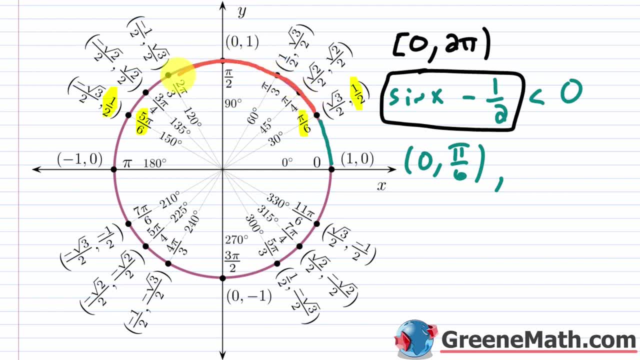 color. so from pi over six, and I'm going to exclude everything again. So pi over six to five, pi over six, both are excluded. So let me write another interval is pi over six to five, pi over six, both being excluded. And then a final interval here you would take from five, pi over six. 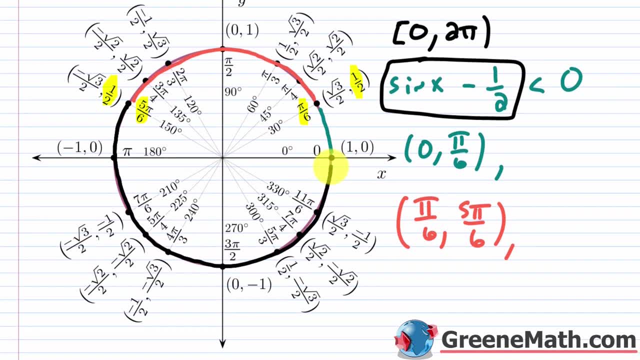 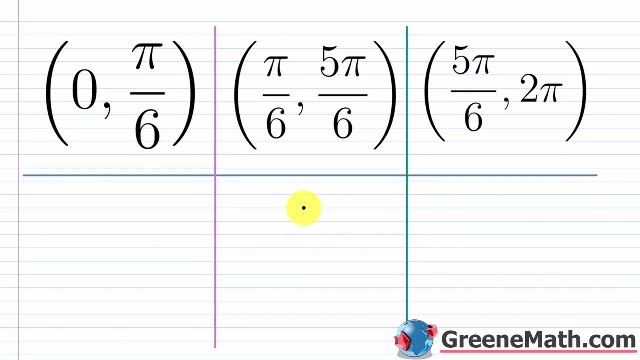 going to two pi again, with both being excluded there. So let's say a final interval would be five pi over six, going out to two pi, both excluded. And I have that written more neatly with a little table. Again, if you want to do that, you can do that in a different way. So let's say: 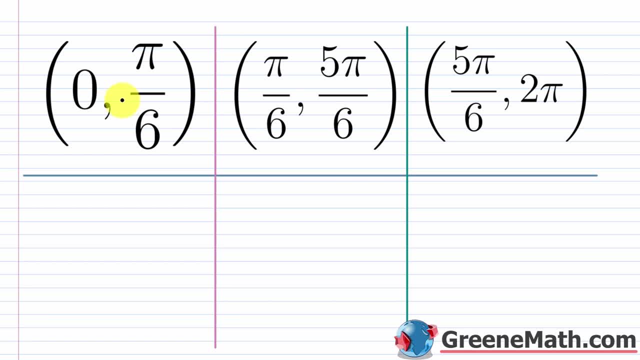 use a number line. it's really up to you. So all you have to do is pick something in each interval and test it and see if it works, So you can say true, false, something like that. You can also just figure out the sign. So, basically, is it positive or is it negative? So, coming back up, 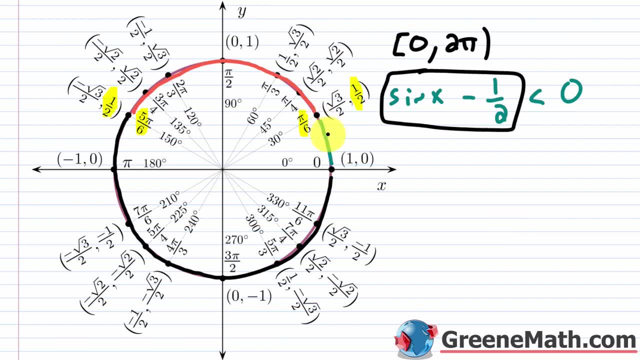 that's really easy to do And this first guy here. so, between zero and pi over six, is this guy going to be positive or negative? Well, basically it's going to be negative, So let me put a negative sign there. And then, between pi over six and five, pi over six, would this guy be positive or? 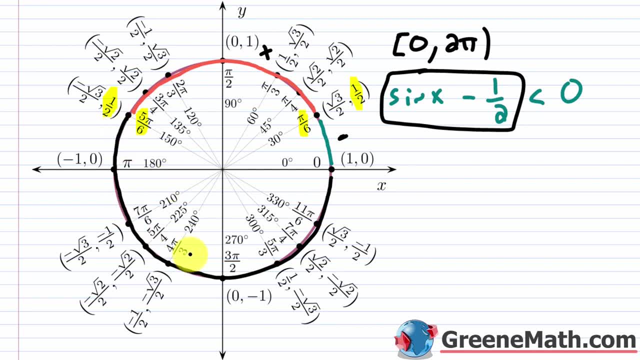 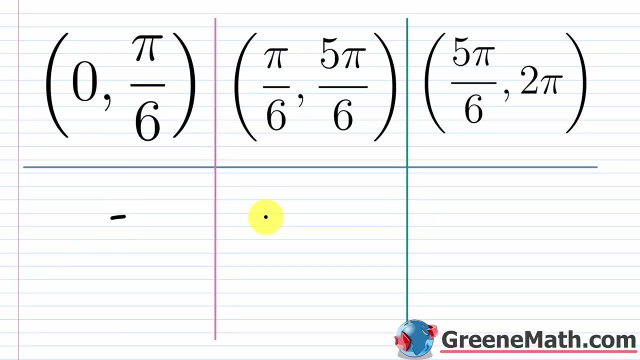 negative. Well, it would be positive, And then in this case it would be positive or negative. This interval right here between five pi over six and two pi, is it positive or negative? Well, it's going to be negative. So, coming back, we want to put that it's negative here, it's positive here. 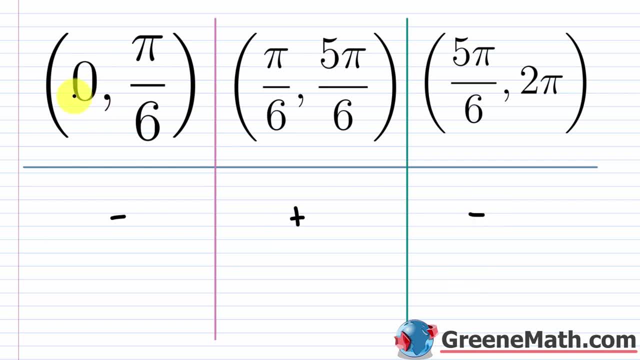 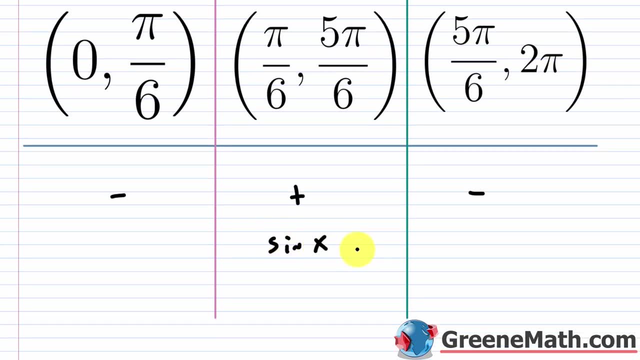 and it's negative here. So if you want to put a solution together, you would say that it's going to work here, it's not going to work here and it's going to work here. In other words, we're trying to figure out where is the sign of x minus one half less than zero. So I'm trying to figure. 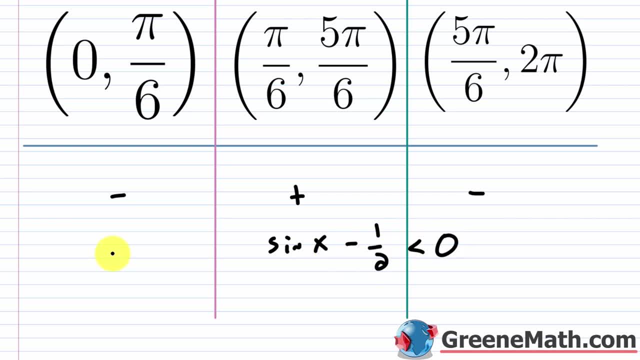 out where it's negative, because that would mean it's less than zero. So here it works. So let me put this in as x minus one half, And then I'm going to put it here. So I'm going to put it here. 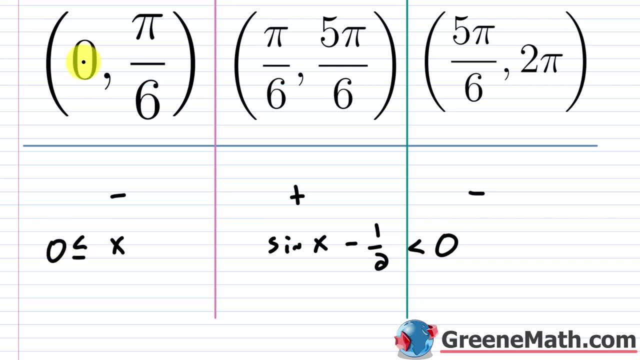 X being greater than or equal to zero. I'm going to go ahead and include zero, because that's in the interval we're solving over Again. when I set up my table, I exclude things, just to make it simple. So x would be greater than or equal to zero and you would have less than pi over six. 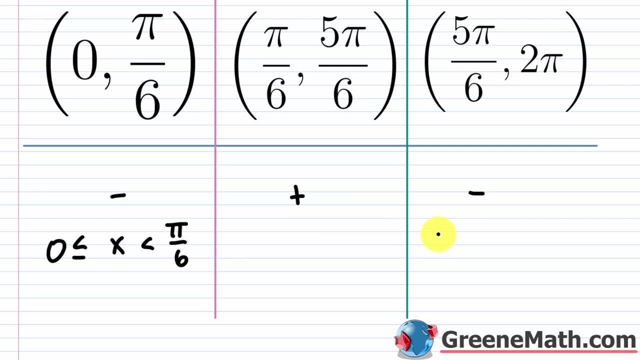 And then this part: right here it's positive. So we don't want that over here. you're going to have this interval, So two pi is excluded and five pi over six. they're both excluded. So you're going to say x is greater than five pi over six and less than two pi. So just put this together, Let. 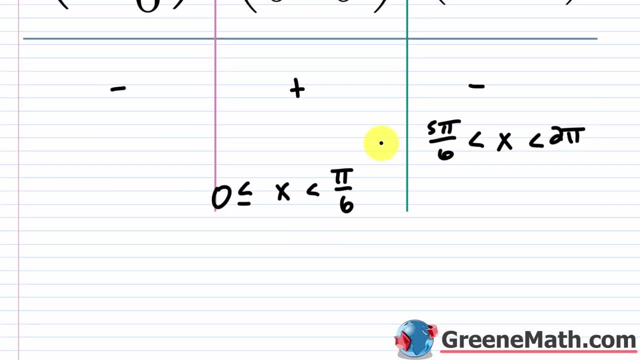 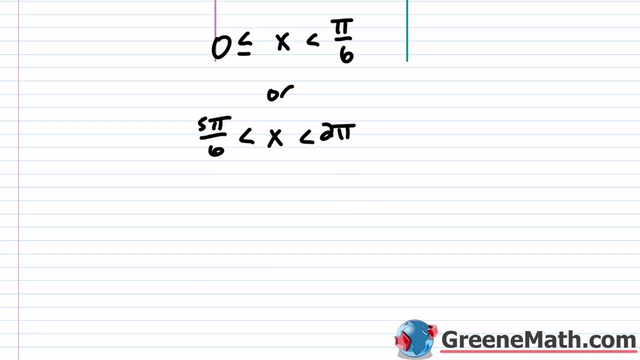 me slide down a little bit. So let me actually just grab this and move it here, and then grab this and move it here And I'm just going to use the keyword, or that's all you have to do. Another way you can do this is you can put it in interval notation, So you can put a bracket with zero. 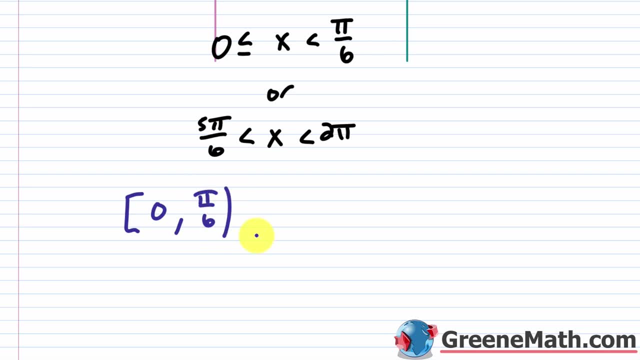 and then you're going to go out to pi over six and that's going to be excluded, So you use a parenthesis. And then the union with you're going to use a parenthesis with five pi over six because it's not included, And you're going to go out to two pi And of course that's excluded. 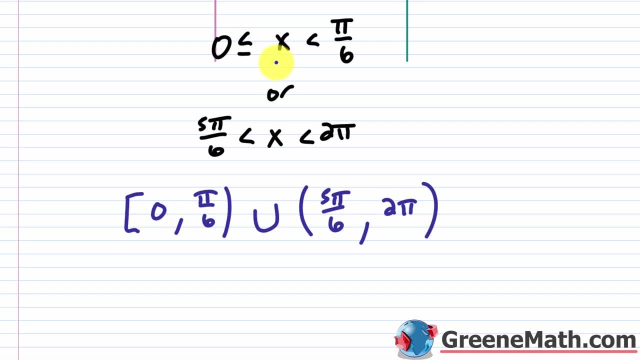 So you're going to use a parenthesis. So this would be your solution: x can be anything that's greater than or equal to zero and less than pi over six, or x can be anything that's greater than five, pi over six and less than two pi. Okay, 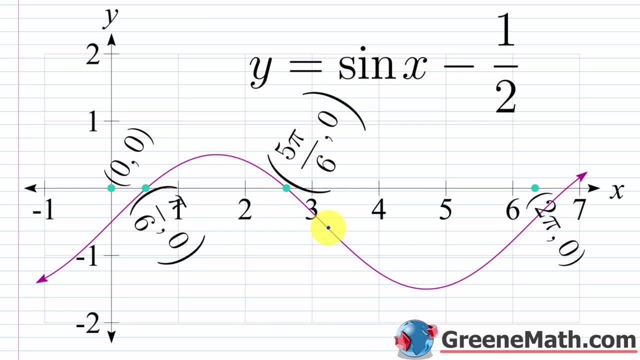 you can always look at these things on Desmos if you're a little bit confused or you want a visual confirmation of your solution. So we have: y equals the sine of x minus one half. remember we were solving: the sine of x minus one half is less than zero. So all I'm doing here is asking where the y. 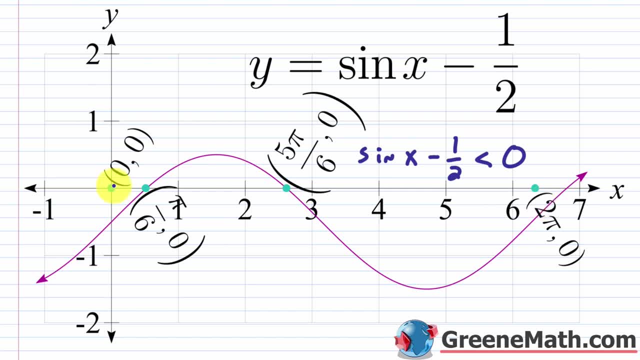 value is going to be less than zero again in that interval that I'm solving over. So if I look at the start of the interval I'm solving over, you can see that you have a y value that's less than zero. So that's going to continue up to the point where you're not at pi over six, So anything less. 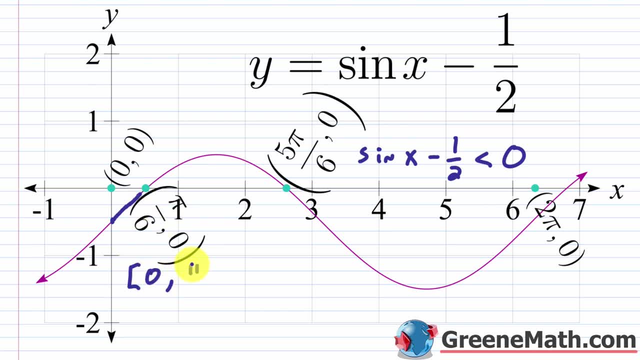 than pi over six. So again, that's where you get the zeros included up to and excluding pi over six. then the union with: if you look at anything greater than five, pi over six- five pi over six itself doesn't work because that's where you're at zero, but anything greater than five pi over. 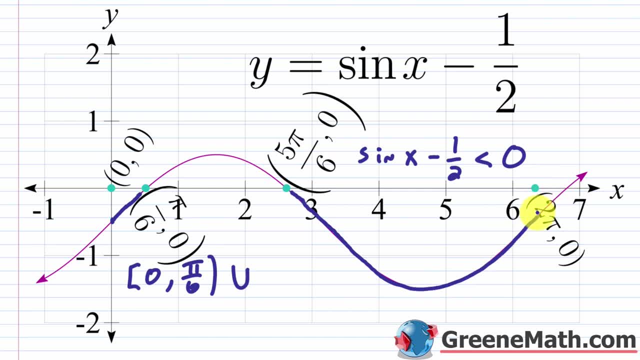 six going up to and excluding two pi, because that's excluded from the interval we're solving over. that's going to work as well. So you put a parenthesis and you're going to get the parenthesis, and again five pi over six and then also two pi with a parenthesis. Okay, let's. 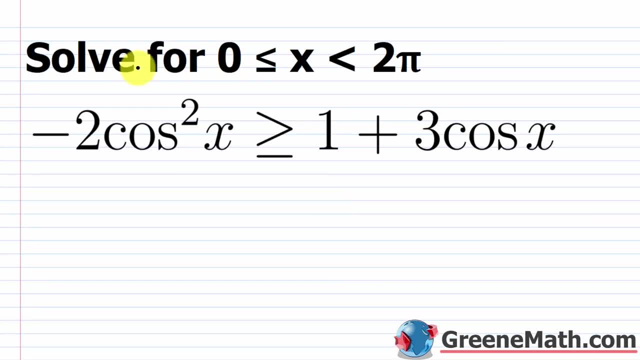 take a look at a problem that's a little bit more challenging. So again we want to solve for: x is greater than or equal to zero and less than two pi, we have negative two cosine squared, x is greater than or equal to one plus three cosine of x. So again I want to make the right side zero In this. 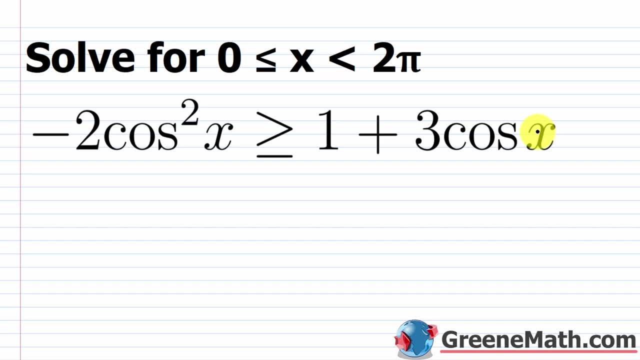 case, I'm going to start off by actually making the left side zero because it's easier, And then I'm just going to switch it around. So I'm just going to add two cosine squared x to both sides of my inequality here. So this right here would cancel and give me zero on the left. So 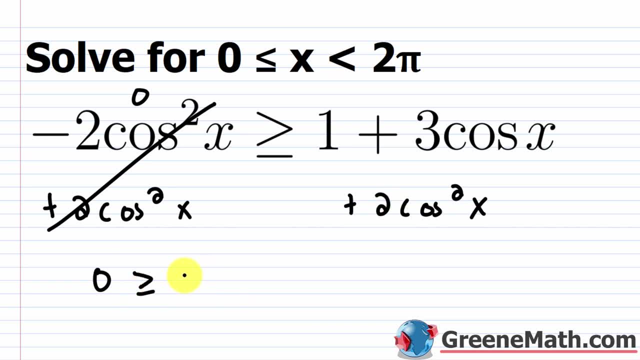 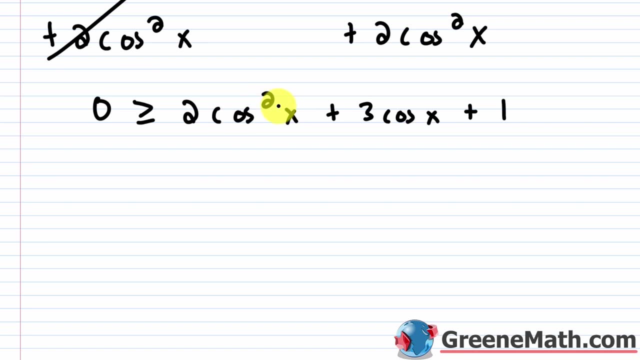 you would have: zero is greater than or equal to. let's write this out in front. So two cosine squared x and then plus three cosine of x and then plus one. Okay, let me slide down here a little bit Now. what I'm going to do is just rewrite this So you can basically say that two cosine squared x. 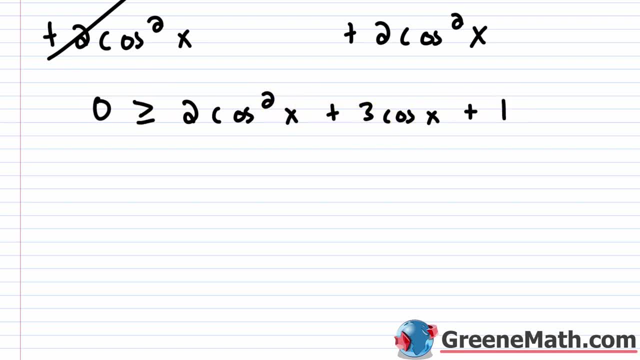 plus three. cosine of x plus one is less than or equal to zero. So that's how I'm going to set, it fine as well. So I'm going to say this is two cosine squared x plus three. cosine of x plus one is less than or equal to zero. All right, at this point you want to find your critical values. 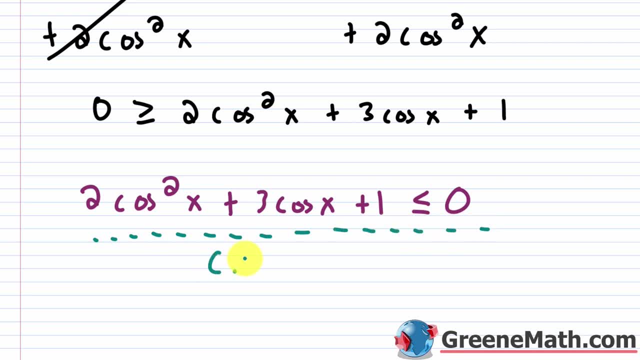 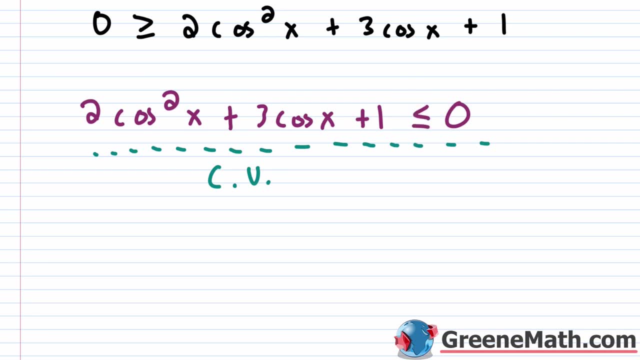 So let me put a little border here and just say that we want the critical values. And again, how do we figure out what the critical values are? Well, basically, you replace this inequality symbol with an equal symbol. So I'm going to solve the equation: two cosine squared x plus three cosine. 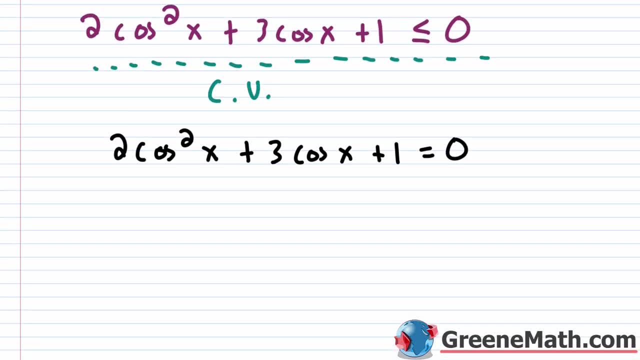 squared x plus one is equal to zero. Now this guy is quadratic in form. So when you get something like this, generally speaking, in a trigonometry class, you can factor it. sometimes you do have to use a quadratic formula, But generally speaking you're going to be able to factor. Let's go ahead. 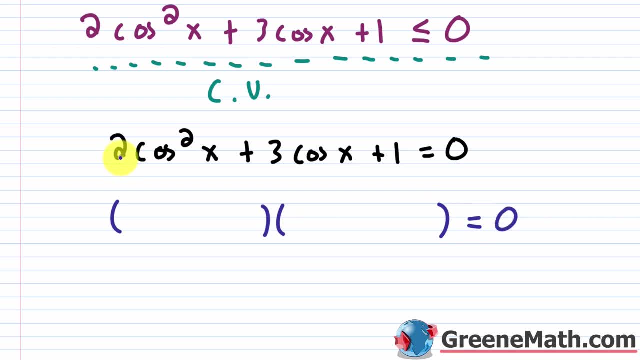 and set this up because we can solve it with factoring here. So this is a two, which is a prime number that tells me this is two, cosine of x And this is cosine of x. So that's easy. The last guy here is a one And this guy is positive. So one is either one times one or negative one. 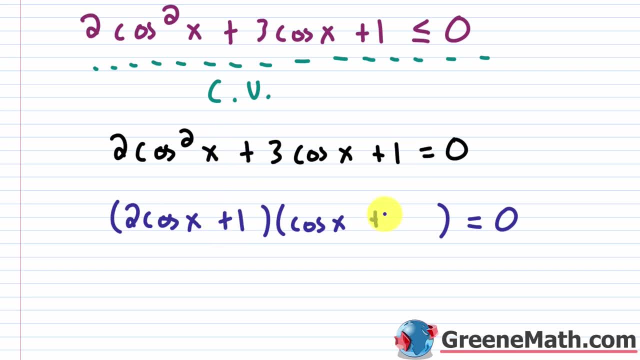 times negative one. But because this guy is positive, I know this guy is positive, So I'm going to do the same thing. I know this is a plus one And this is a plus one. If you want to check it, you do your outer. that's plus two cosine of x, And then your inner is plus cosine of x, So two. 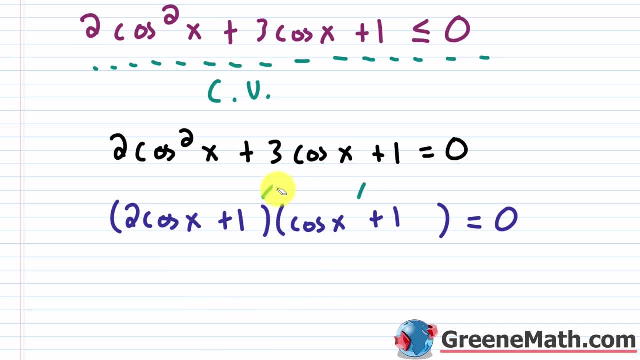 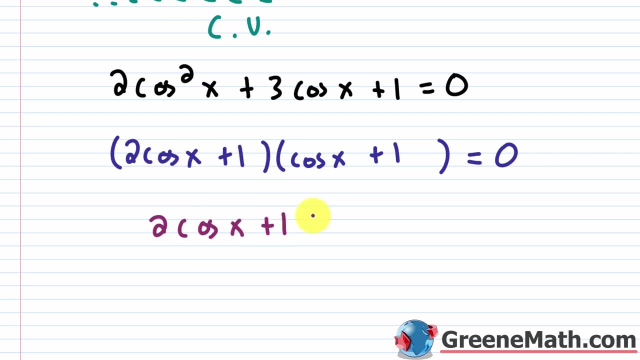 cosine of x plus cosine of x is three cosine of x. So you're good to go with the factorization. So at this point we would use the zero product property. So I would say that two cosine of x plus one. So this factor here set that equal to zero. Let's go ahead and solve that real quick. 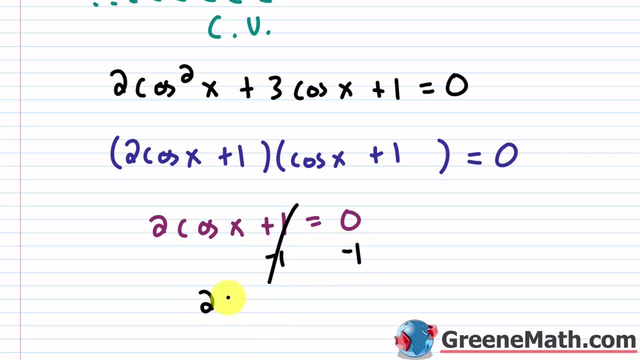 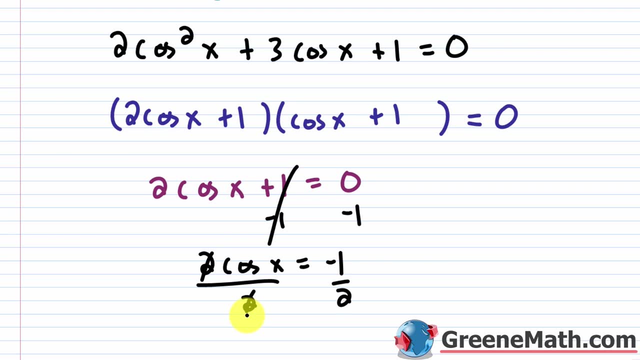 I'm going to subtract one away from each side of the equation. that cancels. you get two cosine of x plus one. divide both sides by two and you're going to get that this cancels. So the cosine of x equals negative one half. let me write that the cosine of x is equal to negative one half And 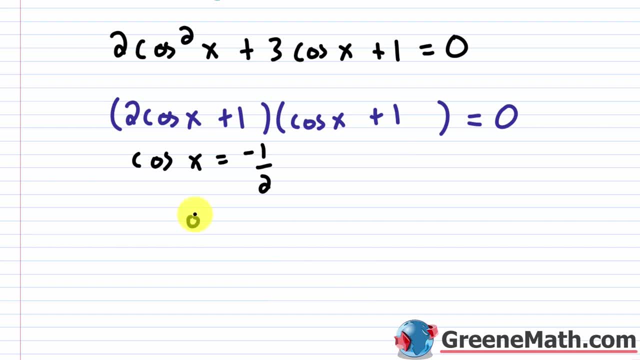 then the other guy is: the cosine of x plus one equals zero. So let me put: or we have: the cosine of x plus one is equal to zero. you can subtract one away from each side of the equation, that cancels, So you get the cosine of x is equal to negative one. So let me grab this real quick And 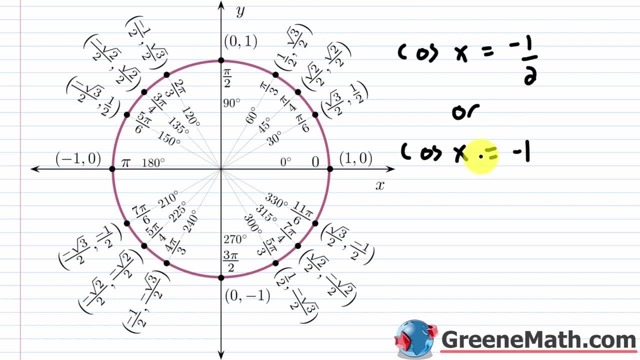 let me come down to the unit circle. So we should get: the cosine of x plus one equals zero. So let's know these off the top of our head at this point. But just in case you don't, we know that cosine is negative in quadrants two and three And I'm just looking for where I have a cosine value of negative. 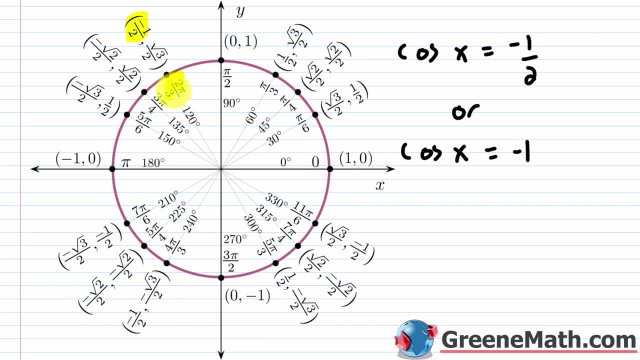 one half. that's going to be right here. So there's your cosine value of negative one half, and that's two pi over three. So then also here's four pi over three cosine value of negative one half. then, for cosine of x being equal to negative one, well, I have a cosine value of negative one. 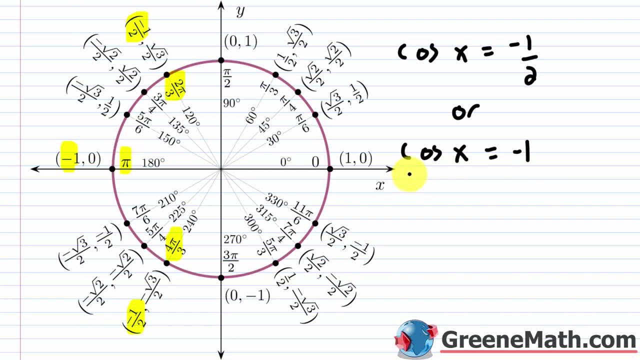 only at pi. So let me put here that we're solving over the interval from zero to two pi. So that's basically. your solutions are: x is equal to you have two pi over three, you have pi, and then you have four pi over three. Now these solutions are the critical values And basically we're using 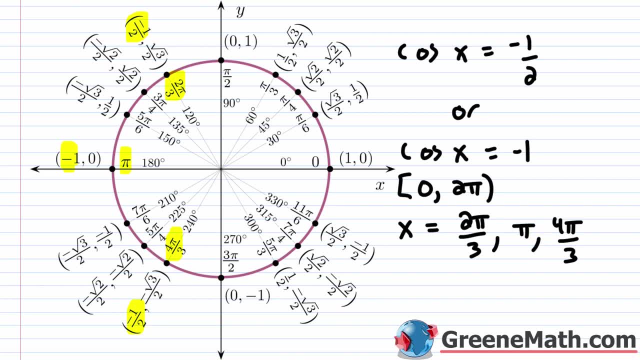 this to split the number line up into intervals. So basically I'm going to exclude everything here. I know a lot of people like to include zero because it's included in the interval that we're solving over. But just to keep things simple, I am going to exclude everything and 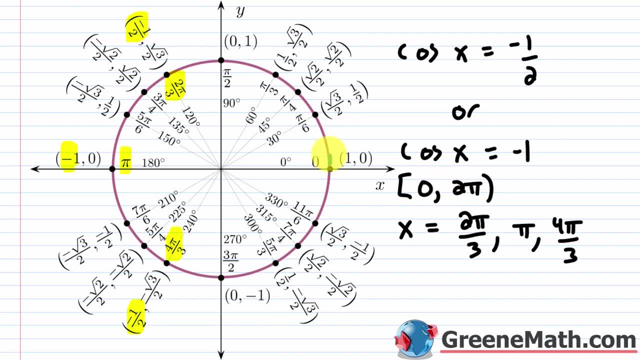 we'll put things together at the end. So for one interval here I'm going to go between zero and, and let's say two pi over three. So that's one interval, then another interval. So we're going to go between two pi over three and pi, And then another interval would be between pi and four pi. 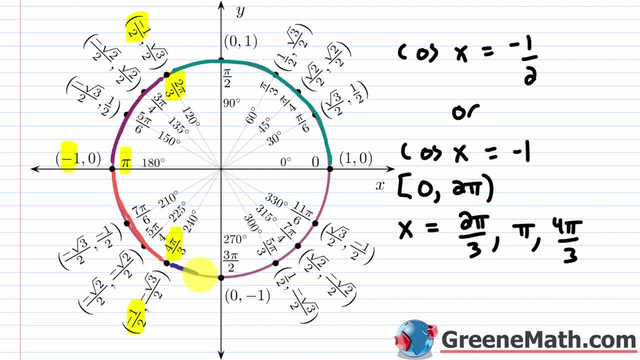 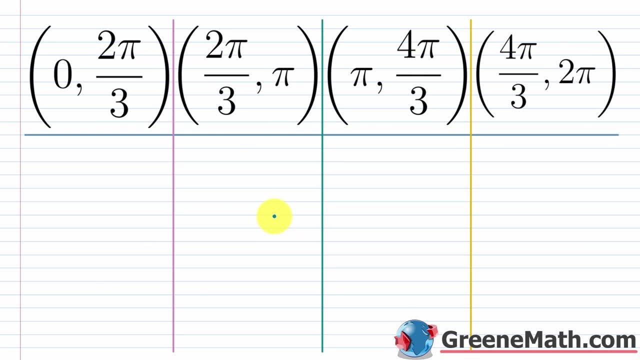 over three, And then for the final interval here we'll say between four pi over three and two pi. So again, I'm not going to include any of those guys, Okay, so once again I'm going to come to a little table. That's what I like to do to organize my information. So you saw that I set. 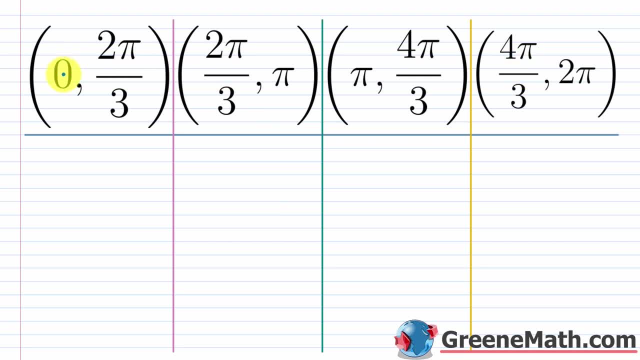 these intervals up on the unit circle. So I have between zero and two pi over three, then between pi and four pi over three, and then between four pi over three and two pi. So when you're testing things, don't ever pick the critical values themselves, Just leave those alone. When we 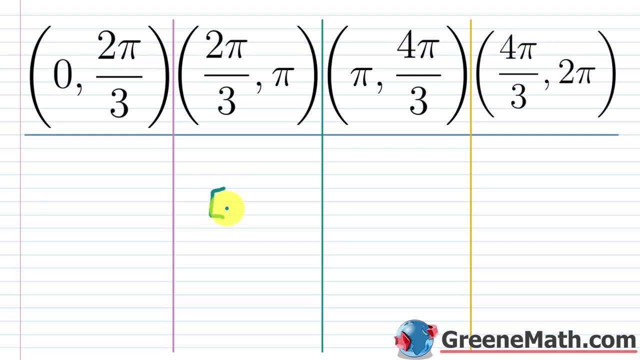 think about zero and two pi. that's coming from our interval. So again we're solving over the interval from zero to two pi, where zero is included and two pi is excluded. And again a lot of you are going to ask: well, why did I not include zero here? You can, if you want This. 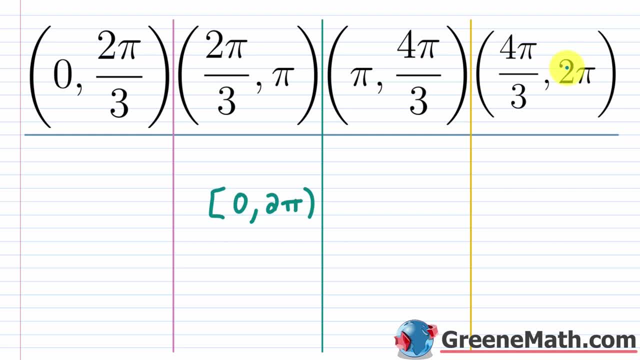 is personal preference. When I set this up, I just exclude everything, And then, once I'm done and I'm putting the solution together, that's where I'm going to think about what's included and excluded. So again, this is up to you. Let me drag this up here out of the way. And then 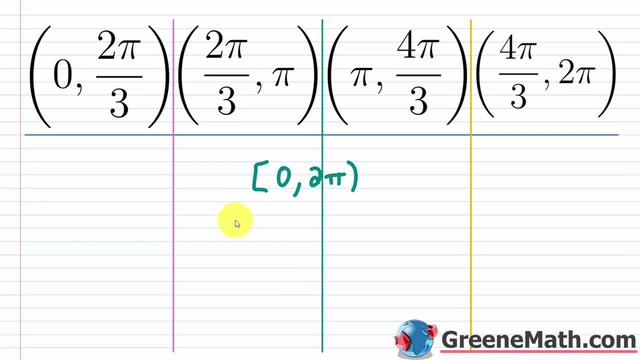 basically I'm just going to write my inequality. So we have two different forms we can use. So the unfactored form is two cosine squared x and then plus three cosine of x, and then plus one is less than or equal to zero. So this is the form I would work with if I was using a calculator Again. 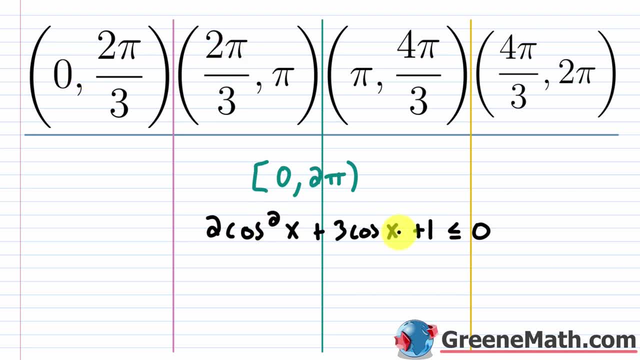 you could just pick something in each interval, plug it in and see if it works, And then the form I would use- if I'm not using a calculator- is the factored form, because it's just easier to work with that if you're not using a calculator. So this was two cosine squared x and then plus three cosine. 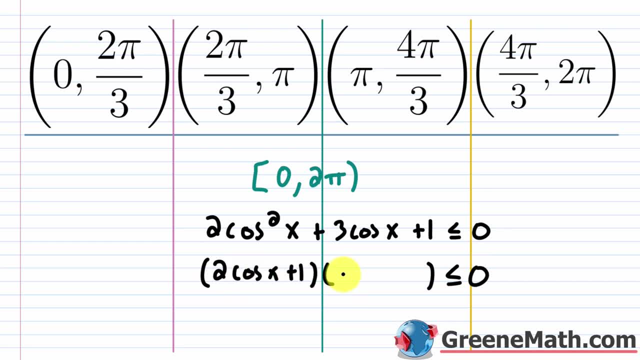 of x plus one and then times the quantity cosine of x plus one. Okay, let me get rid of this unfactored form Again. you can use that if you want. I'm just going to stick with this one. So we know that a positive times a positive, or a negative times a negative is a positive And we 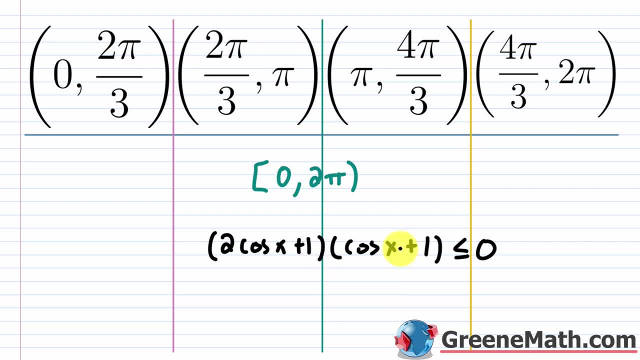 know that a positive times a negative and a negative times a positive would be a negative. I'm going to tell you that this right here, So this right here, this factor based on what we can plug in, is always going to be positive. So I'm just going to put a plus right here. So, basically, 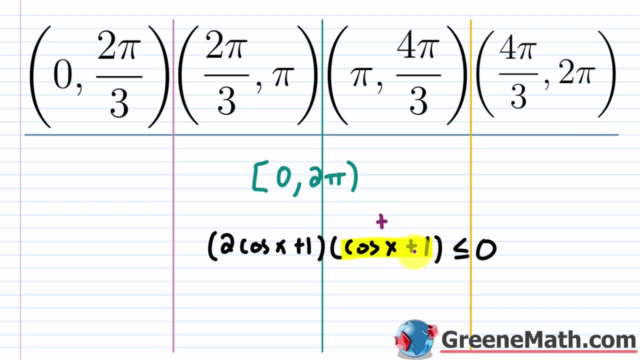 this guy right here is negative, then the whole thing will be negative, And if it's positive, then the whole thing will be positive. Now let me stop for a minute, Because some of you will say: well, why is this factor always positive? I want you to think about the cosine function in general. 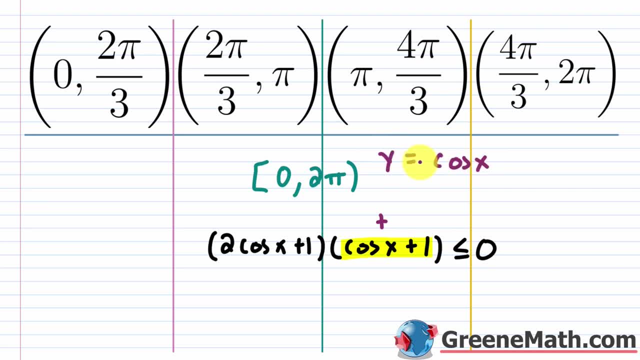 So if you have the cosine of x, or you could write, y equals the cosine of x, the range for that guy, as we know, is going to be from negative one to positive one, And so you get this negative one here when you plug in a pi for x. well, we can't plug in pi here because 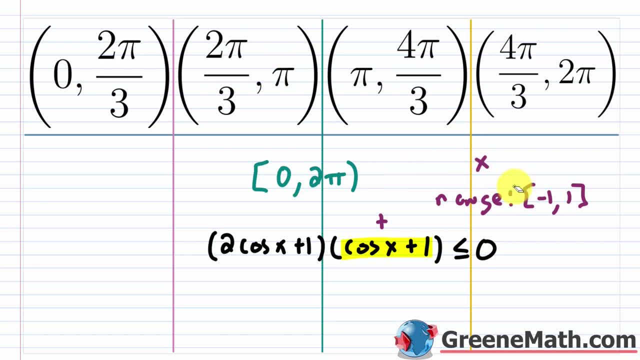 it's a critical value, So you're not going to be able to use that. So, basically, when I think about the cosine of x, well, the smallest I can make this is if I plug in a pi for x and I get a. 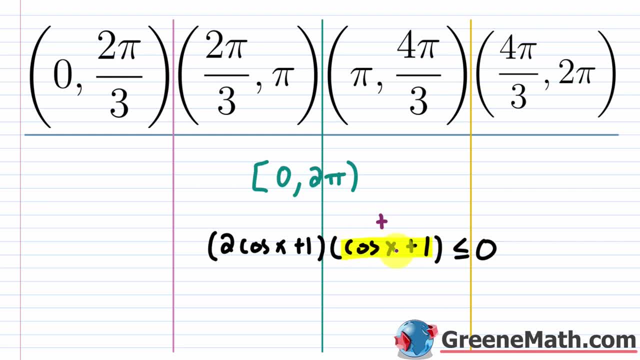 negative one. negative one plus one would be zero. but it's not going to be zero because I can't actually choose pi, So it's going to have to be positive here. So I know that when I look at this factor over here- now I have let me put this as a little border- we have two cosine of x plus one. 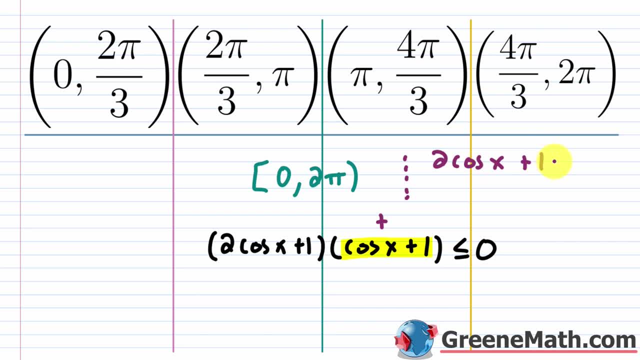 So just ask yourself the question: where would it be negative? solve a very simple inequality for that. So just say: where is this less than zero? subtract one away from each side of the inequality that cancels, you're going to get two cosine of x. 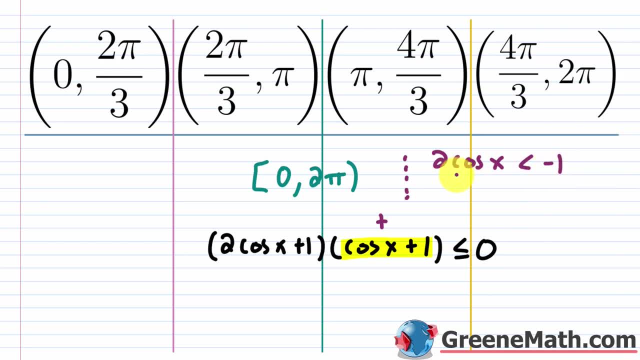 is strictly less than negative one. So this is less than negative. one divide both sides by two, And so basically the cosine of x. if that's less than negative one half, then this right here would be negative, And so the whole thing would be negative And this guy would be satisfied. 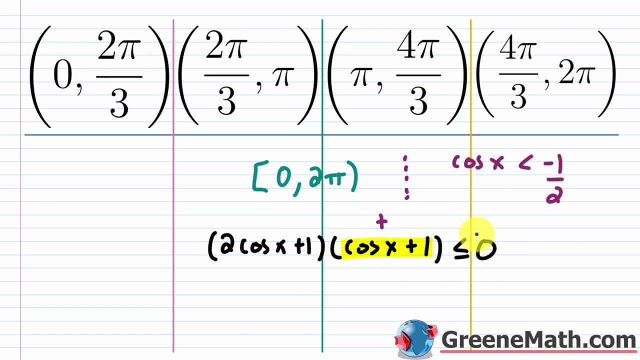 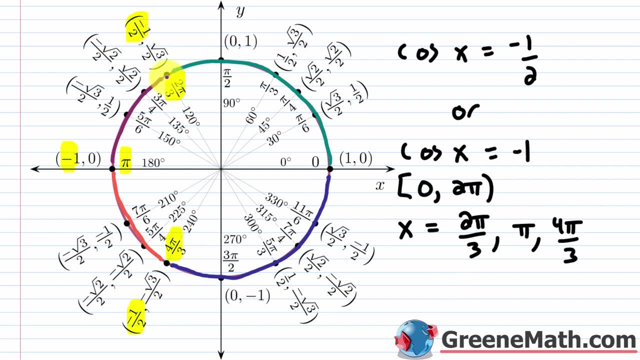 Because if this side right here is negative or if it's zero, we'll have a true statement. So let's see where- hey, why can't I make it up? and see where- the cosine value is less than negative one half. So that looks like this interval right here. So that would make this negative. And then this interval. 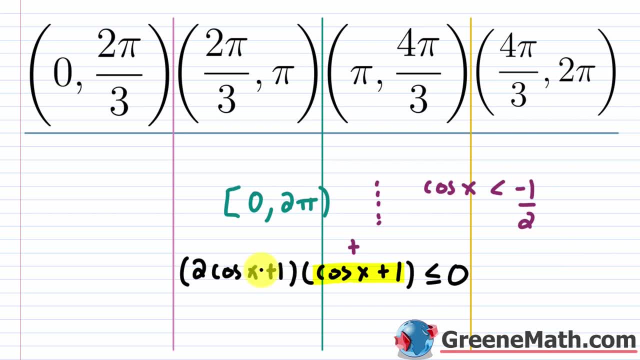 right here, So right here, that would make this negative, Alright. so coming back to the table, we know that this guy right here would be negative And this interval right here, So between two pi over three and pi. and then this interval right here, so between pi and four pi over three. so let 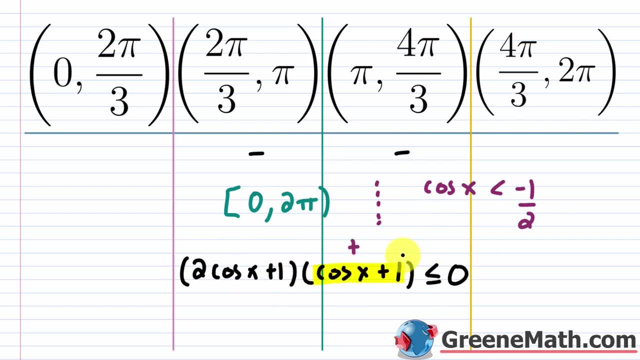 me put that in there, So we would satisfy our inequality there, and that's always going to be less than zero. So in this interval here and this interval here, this factor would be positive, And so the whole thing would be positive, And so that's never. 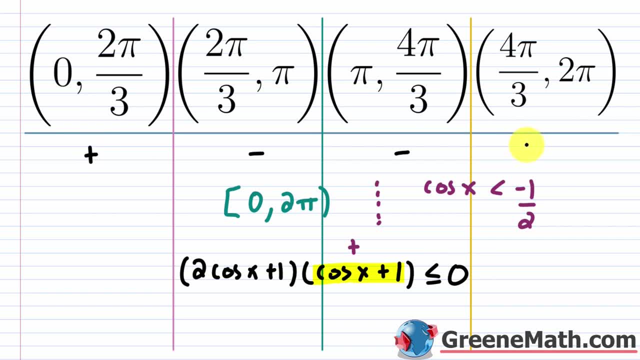 going to be less than zero or equal to zero. you can put a plus here and a plus here to show that okay. so, to put the solution together, you would think about where this works. So, because it's a non strict inequality and we allow for the possibility of this guy to be equal to zero. 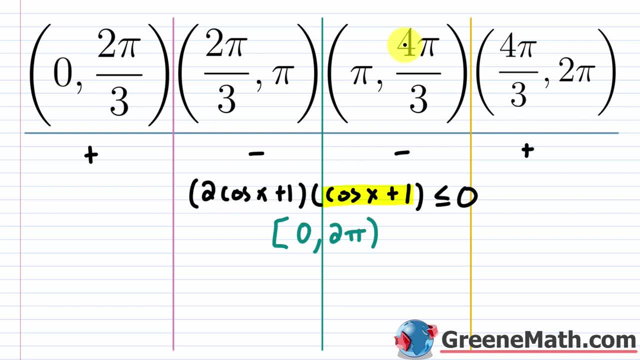 well, two pi over three pi and four pi over three. those are all going to work. So if you started off by just listing these in terms of the table, you could start with: x is greater than or equal to two pi over three and less than or equal to pi, And then say: or you could look at this one, So you 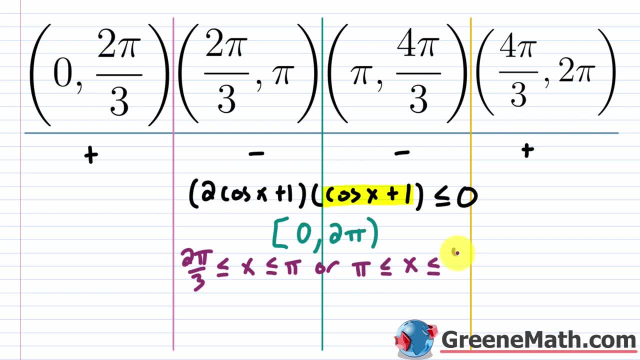 have: x is greater than or equal to pi and less than or equal to four pi over three. Now, of course, you wouldn't write it like this because of the keyword, or what's going to happen is: this is just going to be: x is greater than or equal to two pi over three and less than or equal to four pi over. 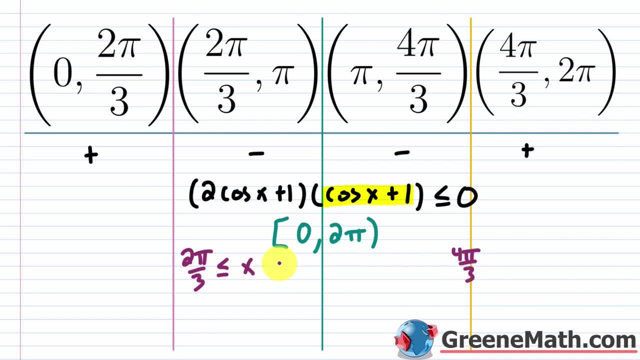 three. So let me tighten this down like this and get rid of that and put a less than or equal to here and just drag this over there like that. So this would be your solution. And if you want to list the interval notation, you're going to put a bracket next to two pi over three and you're 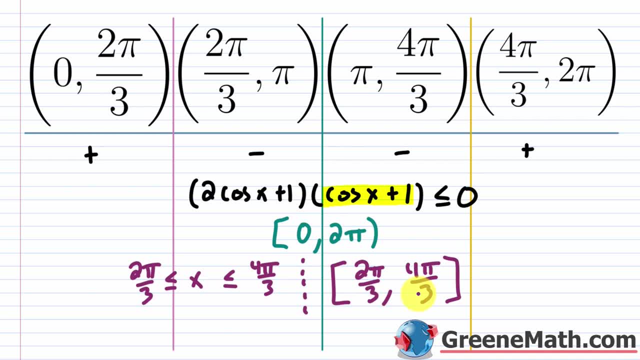 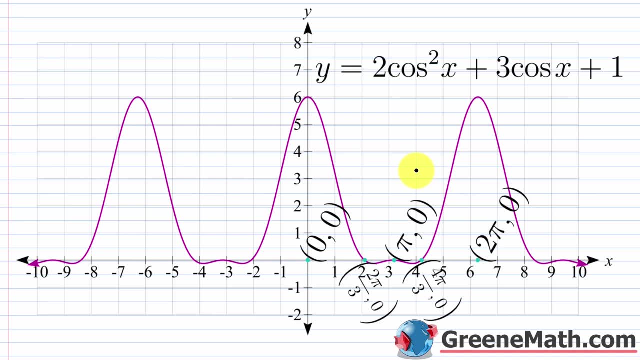 going to go out to four, pi over three, And you're going to use a bracket there as well, because both of these are included. So, once again, if you want to look at this on Desmos, just to get a visual idea of what's going on, you can type in: y equals two cosine squared x plus three, cosine of x plus. 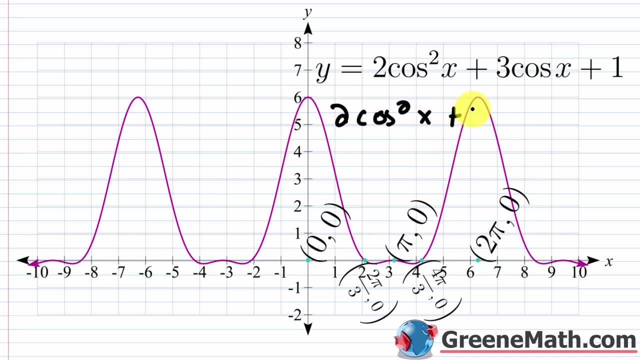 one is less than or equal to zero. So you're basically asking: where are the y values? either zero, so at your x intercepts, or less than zero. So if you look for your x intercepts again, we already know where that's going to be. you have your two pi over three. you have your pi. 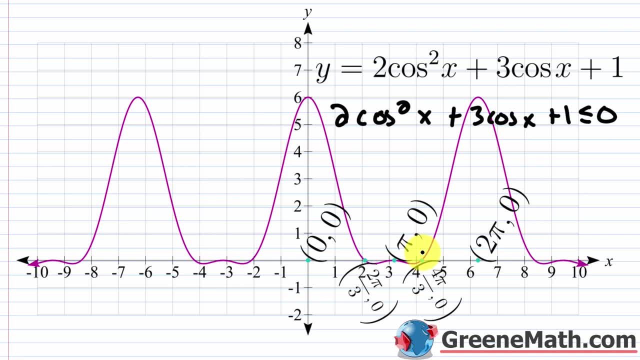 and your four pi over three And then basically you're saying: where is it? either there or less than zero. So you can sketch between these guys and you're going to see it's going to be less than zero. So between those guys. so if you're looking for where it's either zero or less than zero, 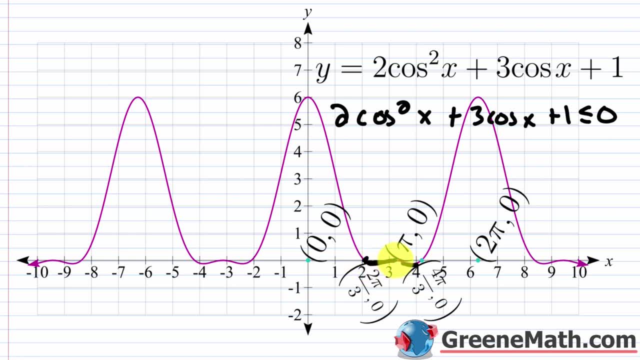 you're going to take this section right here, So from two pi over three, going up to, and including this, four pi over three. that's why we said the solution was again: from two pi over three, going up to and including four pi over three. So that's going to be your solution in the interval that. 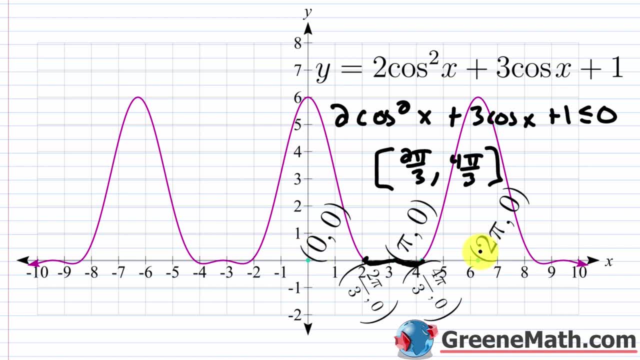 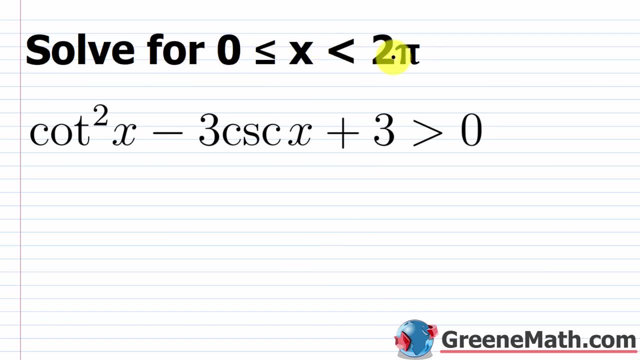 we're solving over from zero to two pi, where zeros included in two pi's excluded. All right, let's take a look at one more of these. So we want to solve for: x is greater than or equal to zero pi. we're given cotangent squared x minus three. cosecant of x plus three is greater than zero. 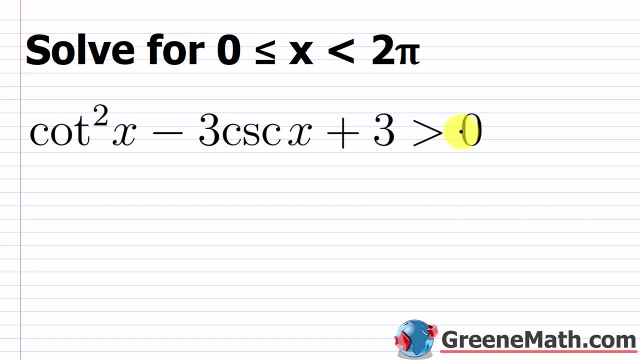 All right. so for this one, we're going to use a little identity to clean things up. you'll notice that the right side is already zero, So we're good to go there. One thing that I would note: if you're working with something that's not sine or cosine, you have to think about where your 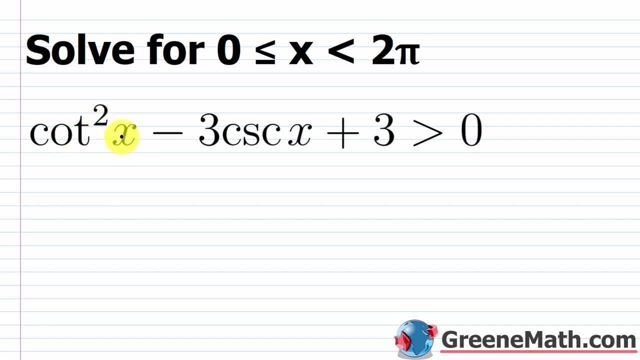 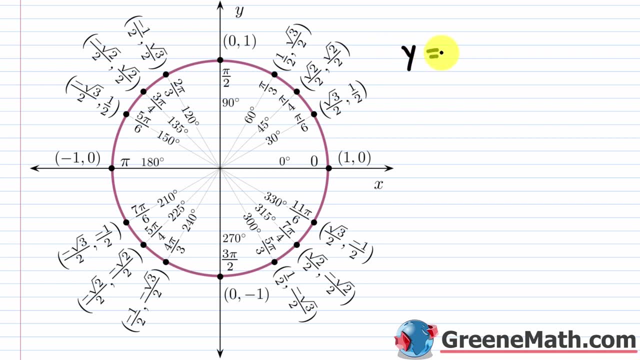 guy is undefined. So if you think about the cotangent squared x and the cosecant of x that you have, let's come down to the unit circle and remind ourselves if you have something like a, y equals the cosecant of x. where is that undefined? Remember that the cosecant of x. 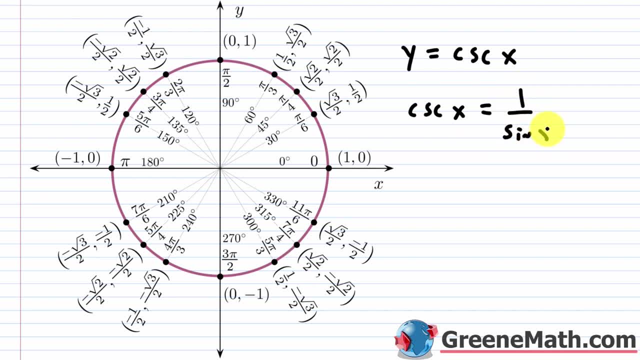 is equal to one over the sine of x. So basically, this guy right here cannot be zero. So where is your sine value zero? it's going to be right here at zero and then right here at pi. So in the interval that we're solving over the x cannot be the angle zero or pi, because again that would 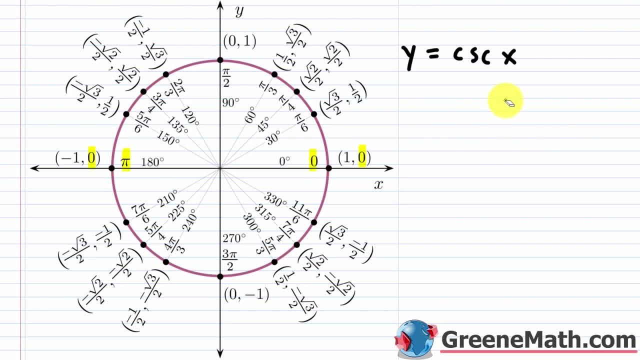 be undefined because you'd have division by zero. So let me put here that the domain, and typically we'll list this by saying that basically it's the set of all x, such that x is not equal to pi, n where n is an integer. So zero pi two, pi, three, pi. 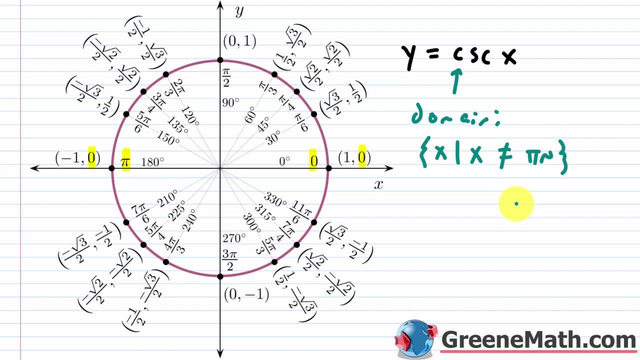 something like that, because again you get division by zero. Then if you think about the cotangent of x, so y equals the cotangent of x and I know we have cotangent squared x, but basically you can extend this to that. Well, when we think about the, 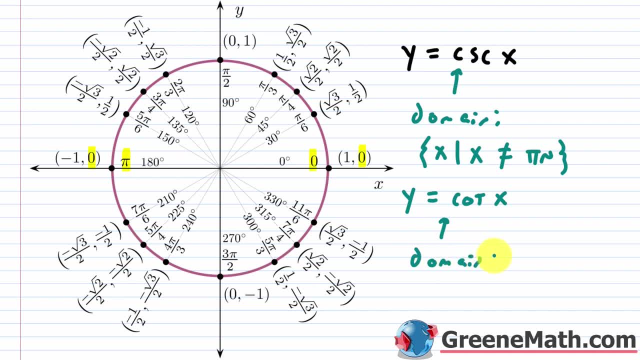 domain here. so what is the domain here? Well, basically it's going to be the same right, because we have the cosine divided by the sine, And so the sine value cannot be zero. So that's going to happen at zero. then pi, then two pi, then three pi, so on and so forth. So 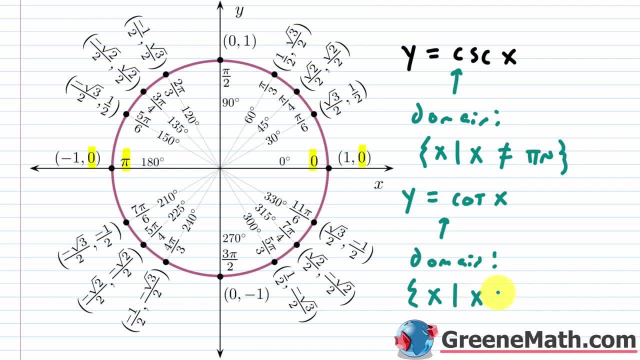 basically it's the same thing. So it's the set of all x, such that x is not equal to pi n where n is any integer. Okay now, if you had again cotangent squared x, the same thing would. 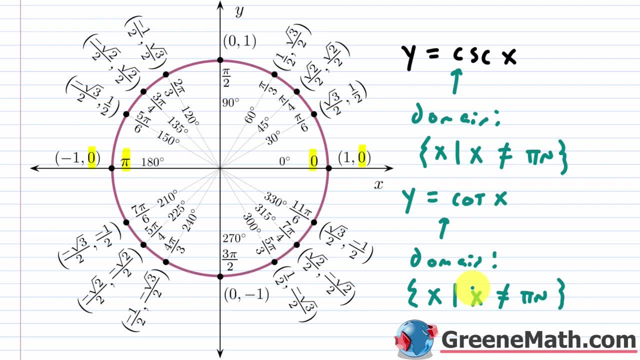 apply because you're just squaring this, so you still can't have division by zero. So that would apply there if you had y equals cotangent squared x. All right, let's get rid of this. we're going to say that at zero and pi, this guy is going to be undefined, So I'm going to keep. 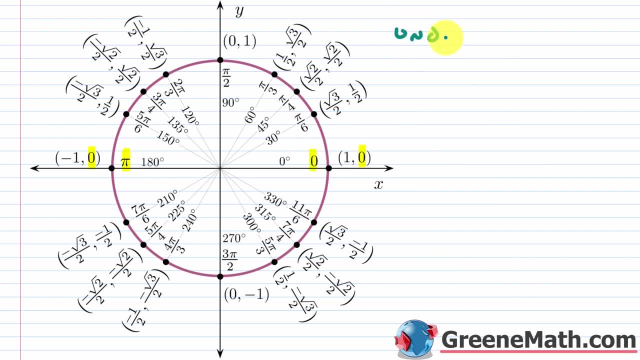 this highlighted for now, And actually we might do better by just saying undefined, So undefined, and just putting a little note here. So I'm going to put zero and pi And that's going to be for in the interval that we're solving over. I'm just going to paste this in here And I have a little. 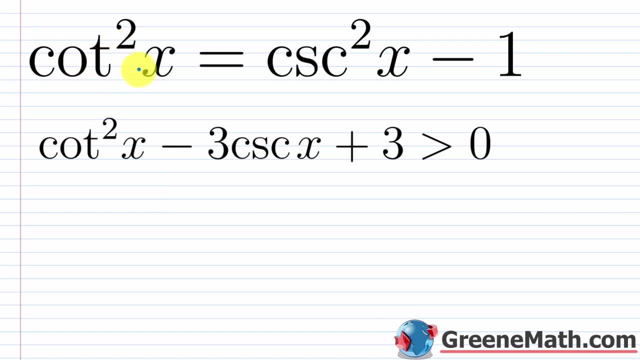 identity set up for us already. So we know that the cotangent squared x is equal to cosecant squared x minus one. So essentially it's going to be the same thing. So we're going to put the this right here matches this right here. So I'm just going to take this right here And I'm going 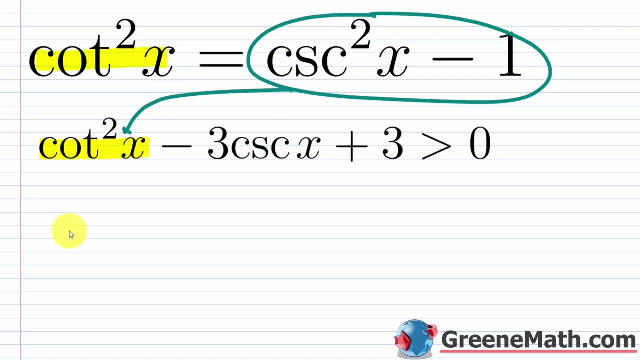 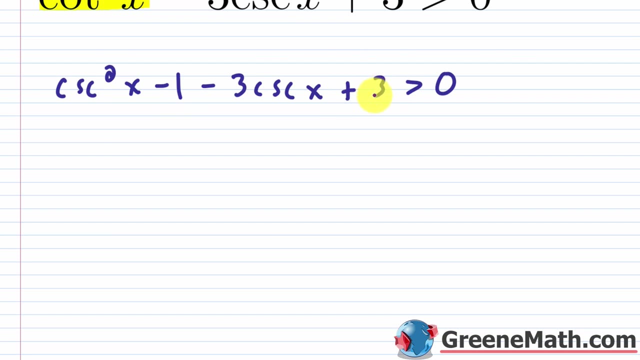 to plug it in for this right here. So that's all I'm going to do. So let's say that we have cosecant squared x minus one- again. this gets plugged in for this- then minus three cosecant of x and then plus three is greater than zero. So you have this negative one and then plus three. 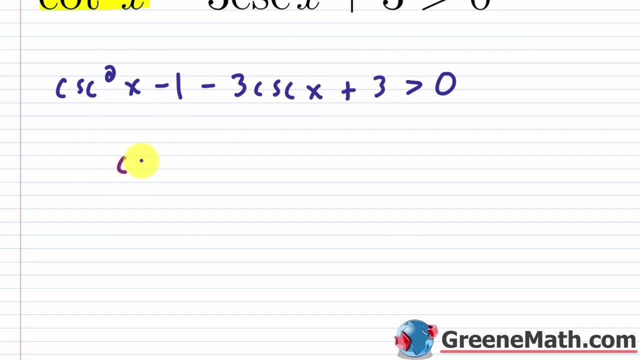 So negative one plus three is positive two. So let's go ahead and write this as cosecant squared x, And then basically plus two, and this is greater than zero. So at this point you would want to find your critical values. So the critical values. Now, this is quadratic and form and you can. 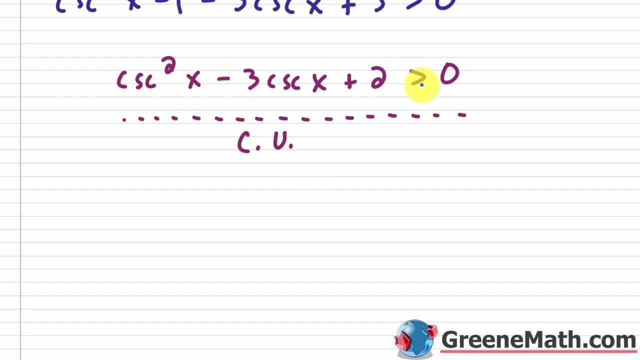 solve it with factoring. So let's go ahead and replace this with equals. So you have cosecant squared x minus three. cosecant of x plus two is equal to zero. Now I would note that, again with the critical values, you're also finding places where it's undefined, And we know that. 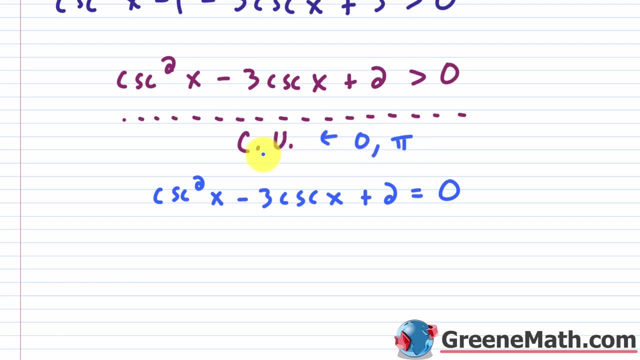 you can put the zero and pi, like we talked about earlier. So you can throw that in the mix now, or you can put it in later, whatever you want to do, But I'm just going to put it in there now So we don't forget. So here, what I want to do is factor on the left. So let me go ahead and set. 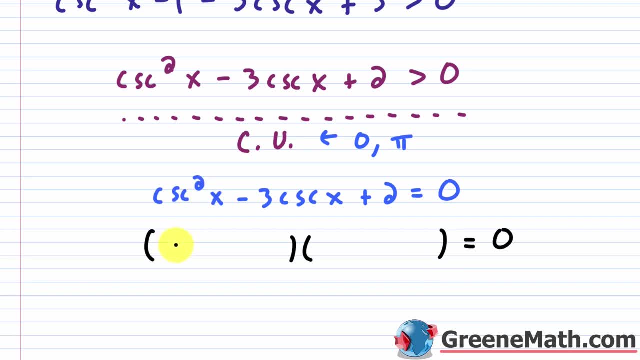 this up with some parentheses. very easy to factor this. So this is cosecant squared x. So it's cosecant of x times cosecant of x. So very easy. This is two, which is only going to come from either one times two or negative. one times negative two. This is negative right here. So 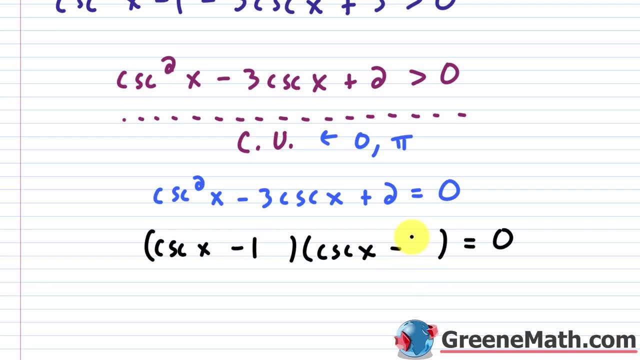 this has to be negative one and negative 2.. Let me make that a little bit better. If you check the outer, here is negative 2 cosecant of x and the inner here is minus cosecant of x. Well, negative 2 cosecant of x. 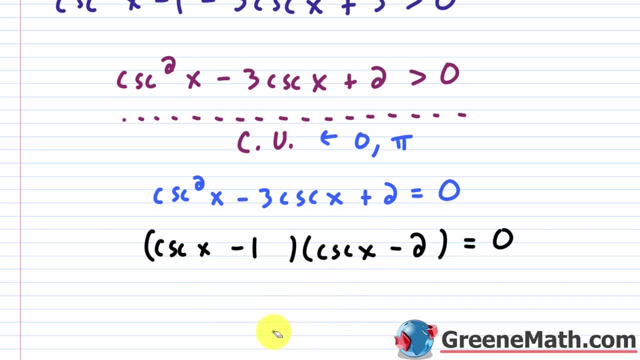 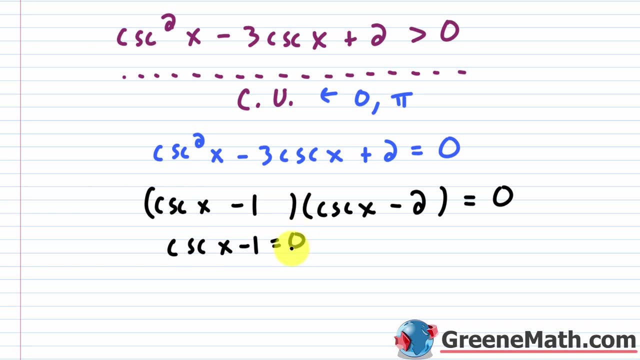 minus cosecant of x is negative 3 cosecant of x. So this is the correct factorization. Okay, let me slide down here a little bit. And essentially you want to find cosecant of x minus 1 equals 0. Add 1 to each side, You get the cosecant of x is equal to 1.. Most of you know. 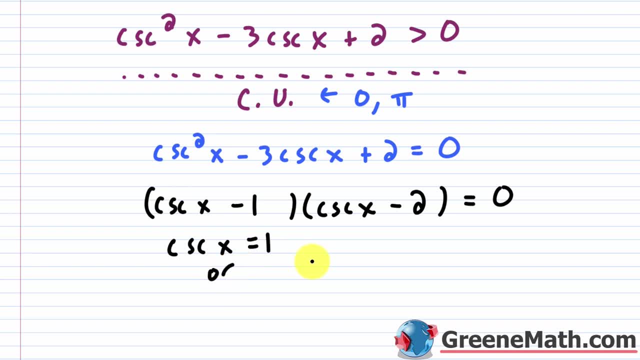 that's going to be at pi over 2, but we'll go to the unit circle in a moment. Then we have: or we have the cosecant of x minus 2 equals 0. Add 2 to both sides, So the cosecant of x. 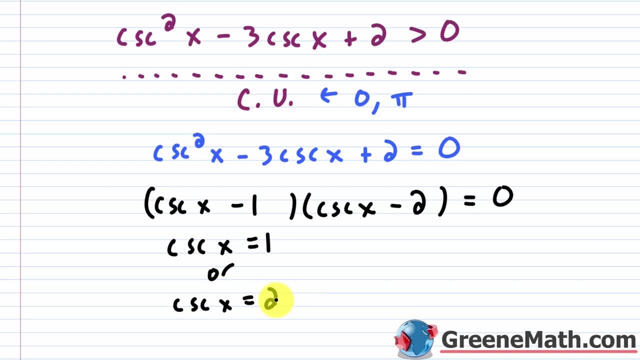 is equal to 2.. So that's going to be at pi over 6 and 5 pi over 6.. Again, let's just go to the unit circle And let me paste this in here, So I have my undefined right there of 0 and pi. 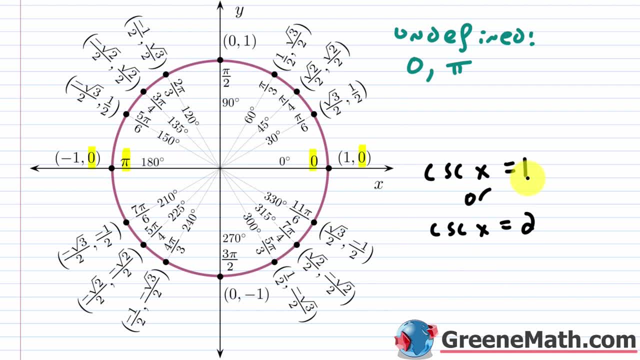 just so we don't forget. So the cosecant of x equals 1.. Again, if you don't know this, you can just convert it over into a sine problem. So we know that the sine of x is equal to 1 over. 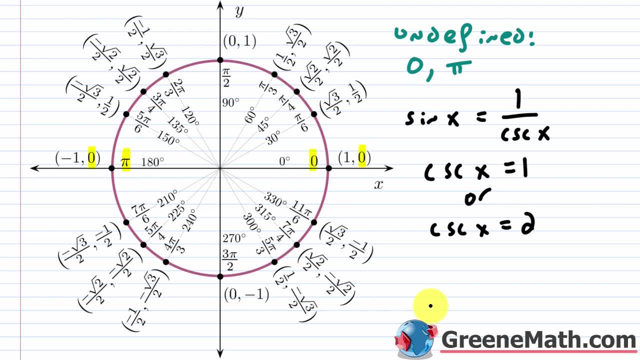 the cosecant Of x. So basically, the cosecant of x is 1.. So this would be 1 over 1.. So where is the sine of x equal to 1?? Well, basically, you're going to be at pi over 2.. That's where your sine value is 1.. 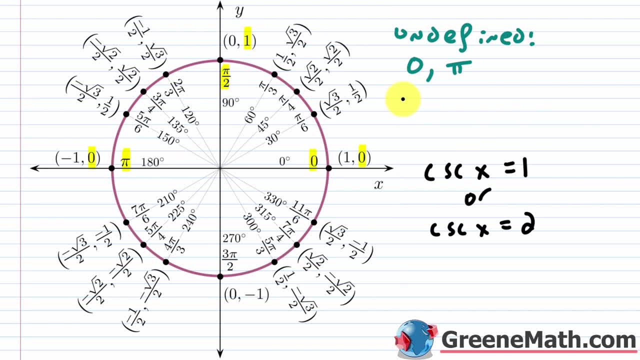 So for that one you can go ahead and say that basically your x is going to be equal to pi over 2.. Now for the other one you have: cosecant of x equals 2.. Again you can convert that over into a sine problem. So you can say that the sine of x is equal to 1 over the cosecant of x. 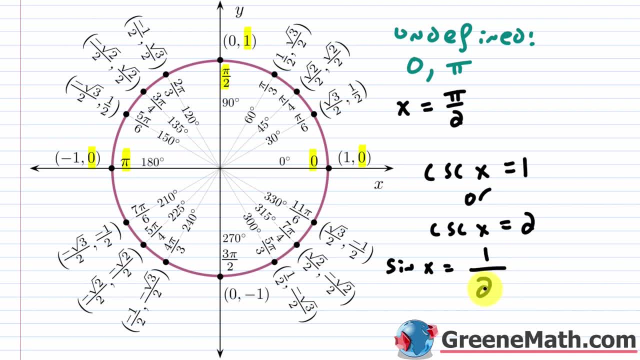 And the cosecant of x is 2.. So the sine of x would be equal to 1 half. And where does that happen? Well, that's going to happen right here, at pi over 6.. And then right here at 5 pi over 6.. Let me get. 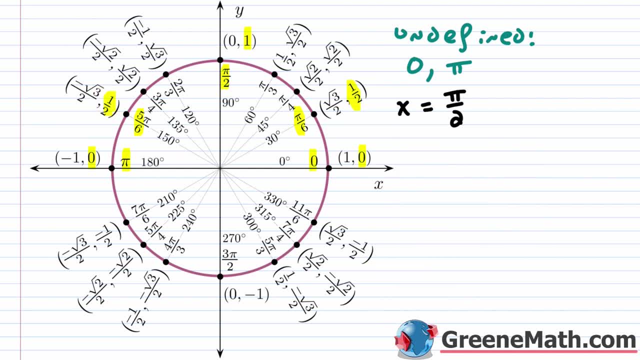 rid of this And actually we don't need this anymore. We can actually get rid of this information. We're just going to list everything out. So, from solving our equation, we have- and I can put this in order, So let's go- pi over 6. And then we have pi over 2.. And then we have 5 pi over 6.. So this: 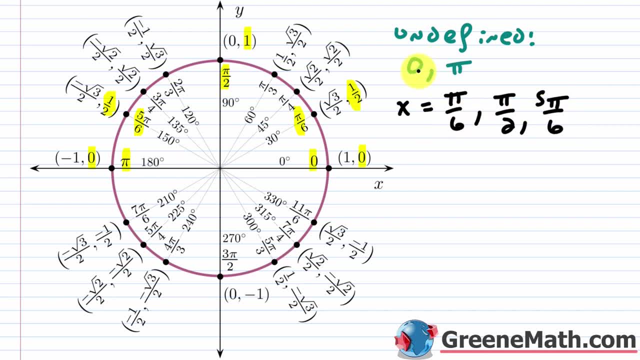 right here comes from solving the related equation. And then this right here, this comes from us determining where things are undefined again in that interval. So basically, you're going to split your- you could say- number line or unit circle again, however you want to think about. 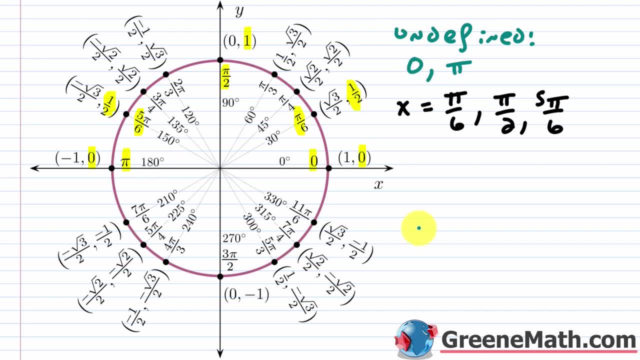 that up into different intervals. So you're going to have one that's between 0 and pi over 6.. So that's going to be this part right here. So you think about something in there. And then the next guy would be between pi over 6 and pi over 2.. So between pi over 6 and pi over 2.. And then you're. 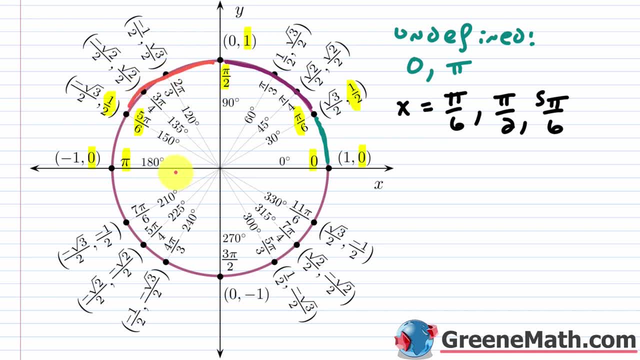 going to do between pi over 2 and 5, pi over 6.. And then you're going to do between 5 pi over 6 and pi. And then you're going to do between pi and 2 pi. So that's the big one right there. In the previous example you saw me use the factored. 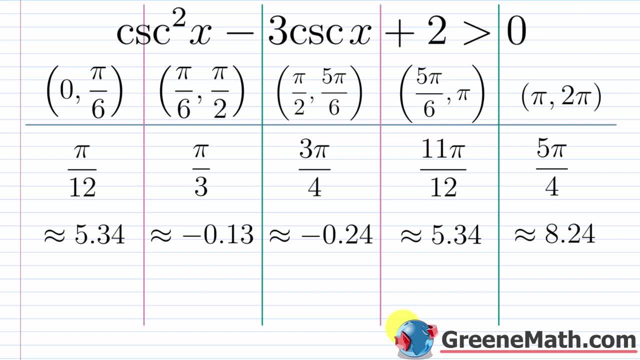 form. But I'm just going to tell you, for something like this, this is going to be very slow if you do that, So you can use the factored form and determine whether it's going to be positive or negative, and do it that way. If I get this type of problem personally, I'm just going to 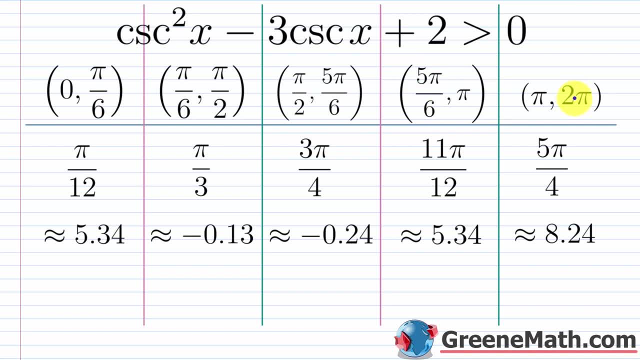 use a calculator, And so I'm just going to go through and set up a little table. This is how I like to do it. Again, nothing will be included here. So between 0 and pi over 6, between pi over 6 and pi over 2, between pi over 2 and 5 pi over 6, between 5 pi over 6 and pi, and then 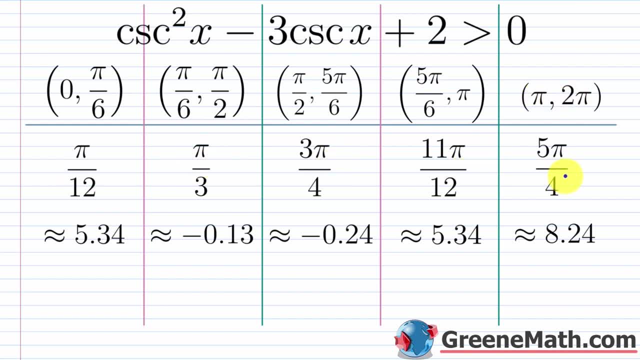 between pi and 2 pi. Now I've already picked something to make this a little bit faster. that's in that interval. You can pick anything in that interval you want, Just don't pick the endpoints themselves, Just pick something between. So I pick pi over 12 here and you punch that. 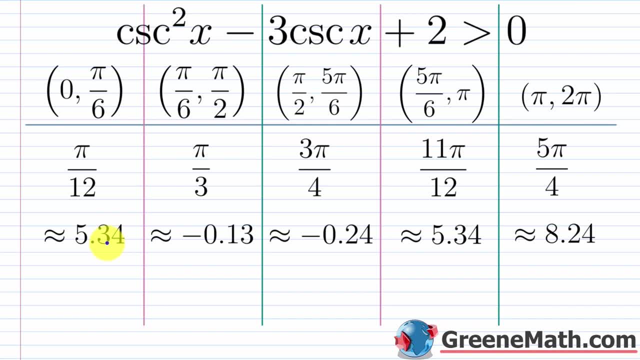 into your calculator, You'll get about 5.34.. Again, I'm rounding this. It doesn't matter, You're just trying to figure out if it's positive or negative. And so this is positive. So, this guy, if you plug in pi over 3, you're going to get something that's negative. So about negative, 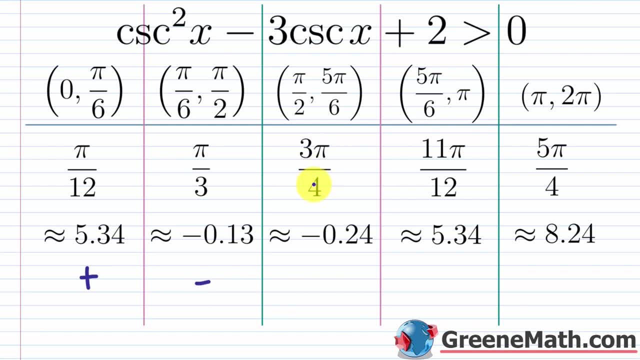 0.13.. So this is negative. here, If you plug in the 3 pi over 4, you're going to get something that's about negative 0.24.. So again, this is negative. And if you look at 11 pi over 12,. 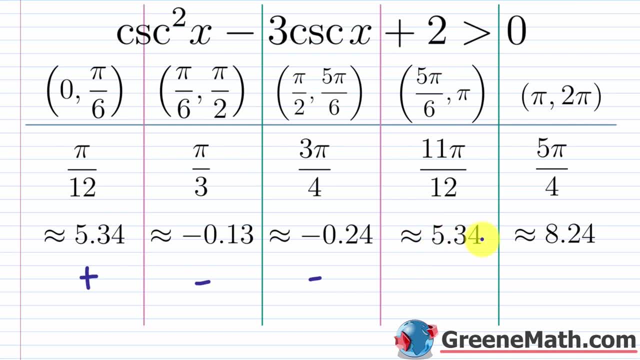 which would have a pi over 12 reference angle. you're going to see that you get that 5.34 again. so approximately, And this is positive. And then, lastly, I'm going to pick this 5 pi over 4.. 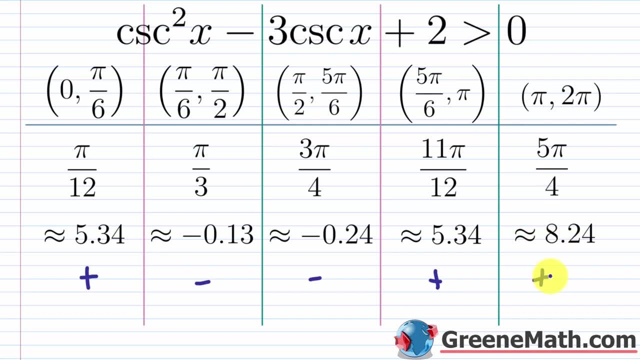 If you plug that in, you're going to get about 8.24.. So this is positive. So we want to know where this guy is greater than zero. So anywhere where it's positive, we're good to go. We have to. 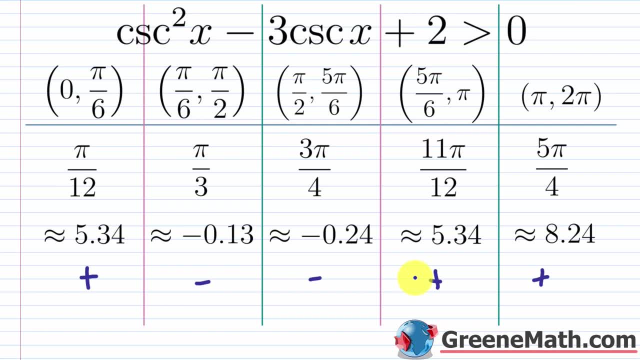 be very careful about our endpoints here, So we know that they're not going to satisfy the inequality in terms of where this guy is zero. But you also have to be very careful about where things are undefined. So that's where this gets really, really tricky. So let me come down here. 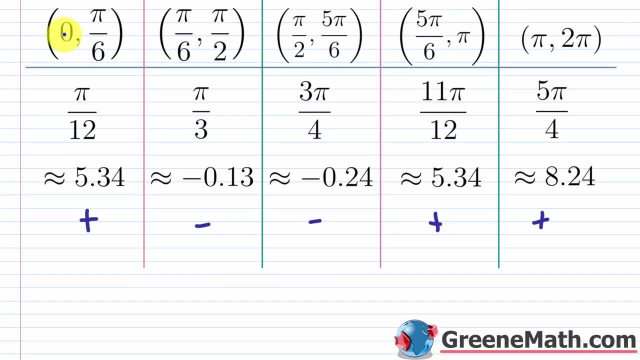 and let me guide you through this so that you don't make a mistake. So you could say: between zero and pi over 6, this guy's going to work because it's positive. Do I want to include pi over 6?? No, because that would make it zero. So that doesn't work because it's a strict inequality. 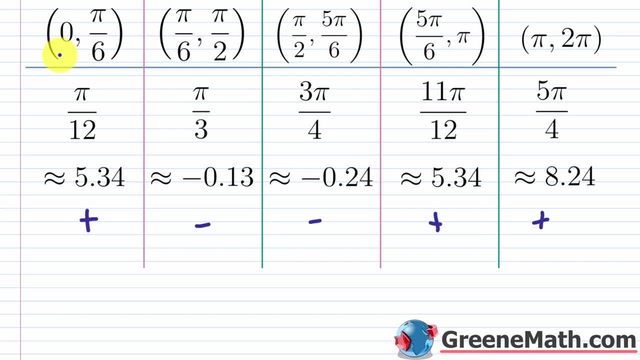 Does zero work? No, because that's where it's undefined. So again, normally you're solving from zero to 2 pi And basically you would include zero and exclude 2 pi. But here zero is where you're going to be undefined, So you have to exclude that there. That's why I never 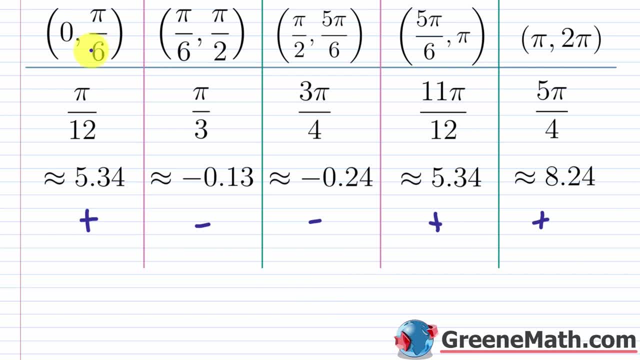 include zero. when I do these types of problems And people always complain. But then you run into a situation like that And you maybe have zero included or something like that. You're not thinking about it And then you get the wrong answer. So that's why I exclude everything, all. 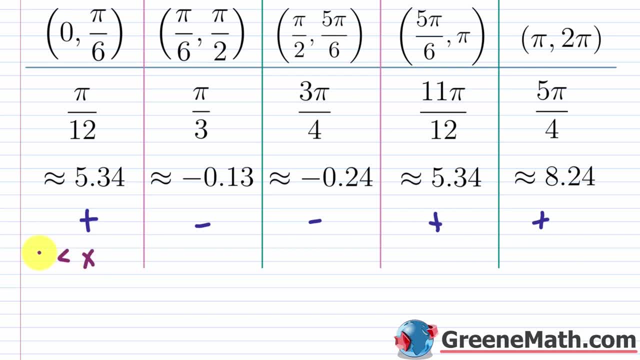 the time. So basically, for this one you would say that x is strictly greater than zero and less than pi over 6.. So neither would be included. Skip this one and skip this one. Now you have between 5 pi over 6 and pi. Would 5 pi over 6 work? No, because it makes it less than pi over 6.. 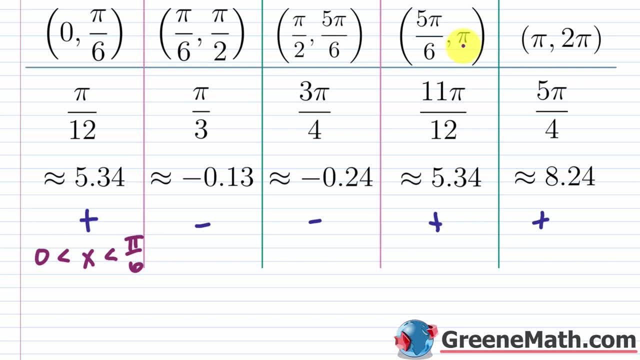 And that wouldn't be included. It's a strict inequality. Would pi work? No, because in this case it's undefined at pi, So it's undefined at zero pi, 2, pi, all those things. So basically this is: x is greater than 5, pi over 6 and less than pi, So it can't be pi itself. So then over. 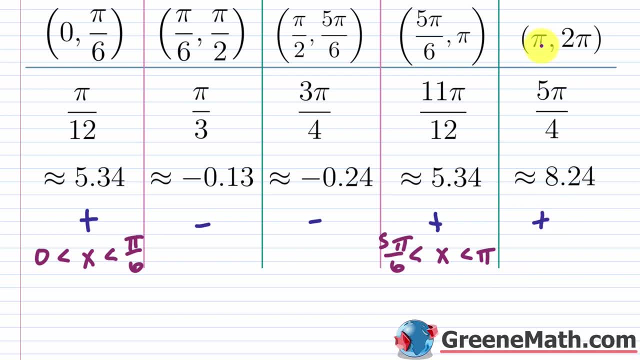 here you're going to have a positive again, But once again pi cannot be included and 2 pi cannot be included. So you're going to say that x is greater than pi And it's going to be less than 2 pi. Now let me put the keyword. 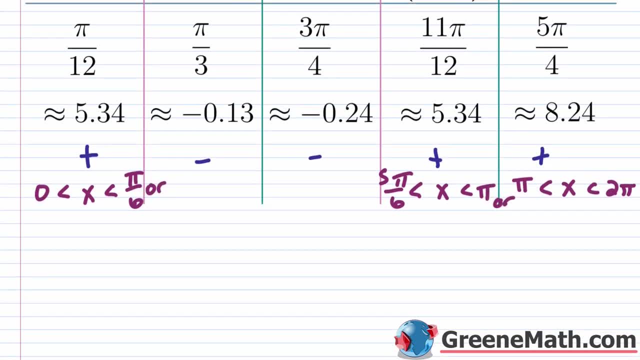 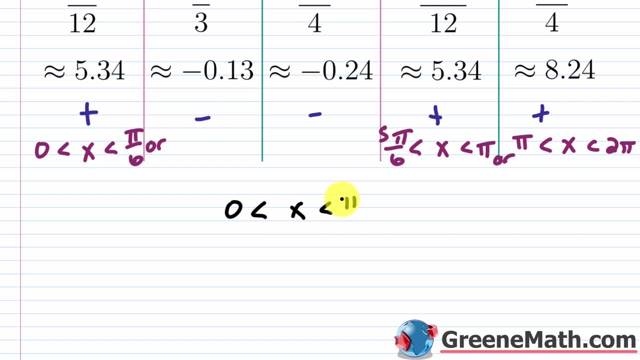 or in here I'm going to try to squeeze that in everywhere. And then let me come down here and write this more neatly, in case you're trying to put this down for your notes. So basically, x is greater than zero and less than pi over 6.. Then you're going to say, or So you're going to. 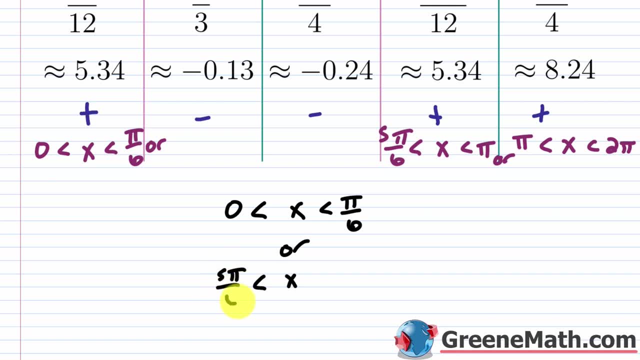 say that x is greater than 5, pi over 6 and less than pi. Now this is strictly less than here, So you cannot combine those two, like a lot of people want to do. Pi cannot be included because it's undefined at pi, So don't put that in there. Let me come down here a little bit and say or: 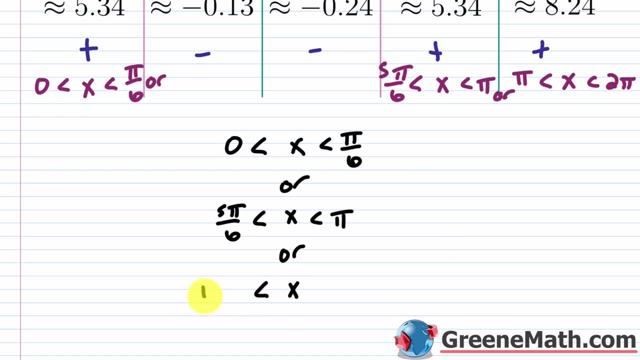 So we have another one of those. We'll say x is greater than pi and less than 2 pi. So that's kind of a lot. But when you solve an inequality like this, sometimes it gets ridiculous. And if you solve one, that's harder, sometimes it gets really ridiculous. If you want to do the interval, 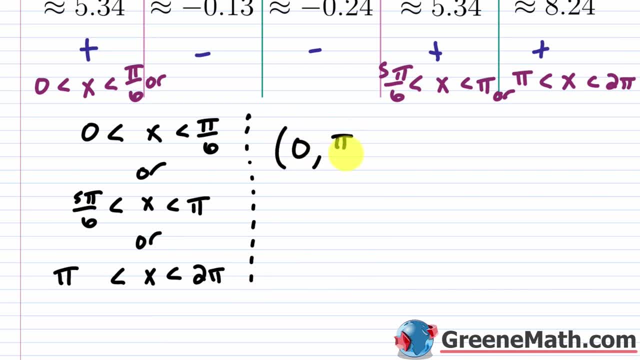 notation, it's not that bad. So you're going to say from zero to pi over 6.. Again, both are excluded. And then the union width you're going to do from 5 pi over 6 to pi. Again, that's both. 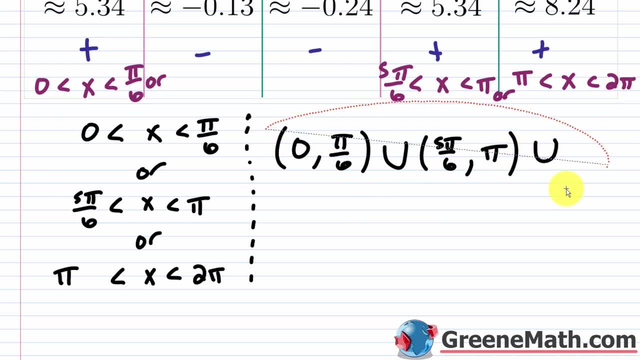 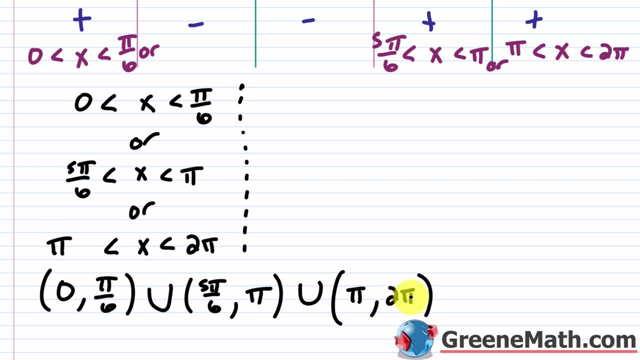 going to be excluded. And then the union width. it looks like maybe I can't fit this, Let me drag it down here, So maybe I can fit it. So the union width: down here you would go from pi to 2 pi. Again, both are excluded, All right. So once again, if you want to go to Desmos and see, 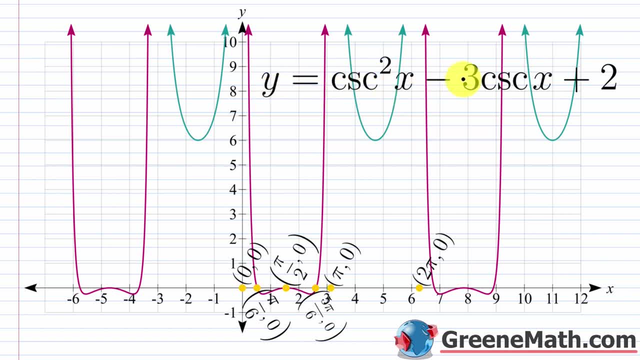 this visually. you can type in: y equals cosecant squared x minus 3, cosecant of x plus 2.. And you'll visually be able to see all the things that I was talking about. So basically, you're asking where's this guy going to be greater than zero? So where are the y values greater than zero? Well, 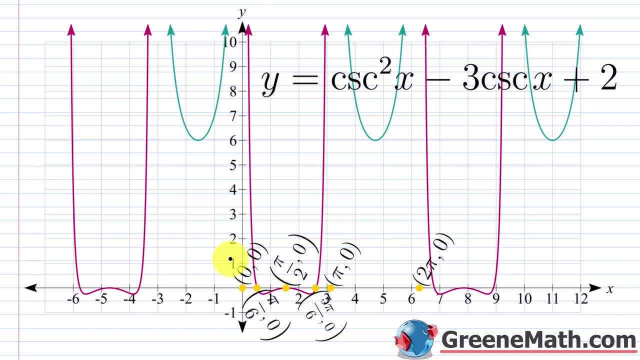 if you start here at zero, notice that this guy can't be zero Because, again, if you plugged in a zero here, this is going to be undefined. So anything that's greater than zero is going to work And this is going to be going up to, and then excluding 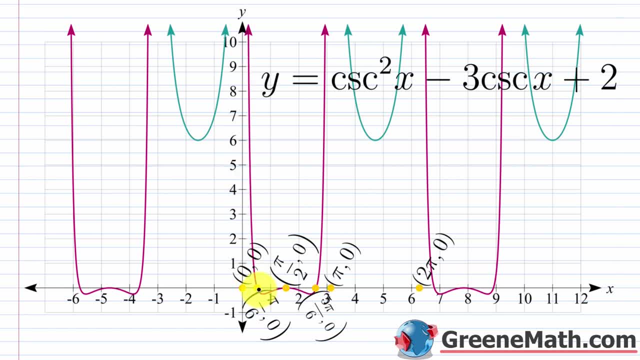 this pi over six. So when you hit pi over six this guy's actually going to be zero. So that would be excluded. So that's where you're getting that zero to pi over six, with both excluded part And then the union width. if you look at it here, I'm going to be below zero at zero, below zero at. 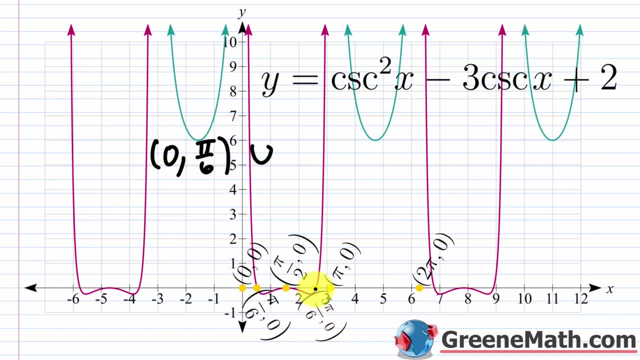 zero. So once I get to five pi over six- I know that's hard to read, That's another x intercept that we found- And basically anything greater than that, going up to an excluding pi, we're going to be above zero again. So we're going to say five pi over six going out to pi. 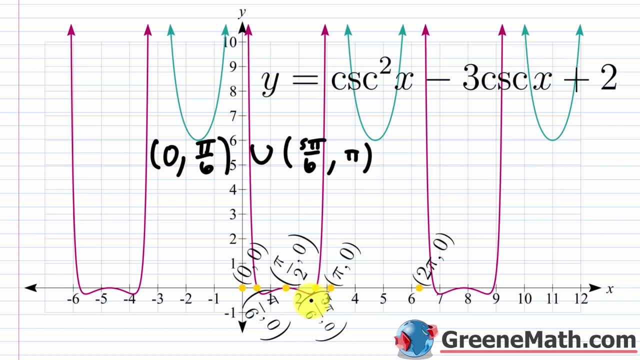 but pi, of course, will not be included, Because you can see that this guy is going to have a vertical asymptote at x equals pi. right, these guys are going to approach an x value of pi, but it won't be able to actually touch it because it's undefined there. So then you have the union. 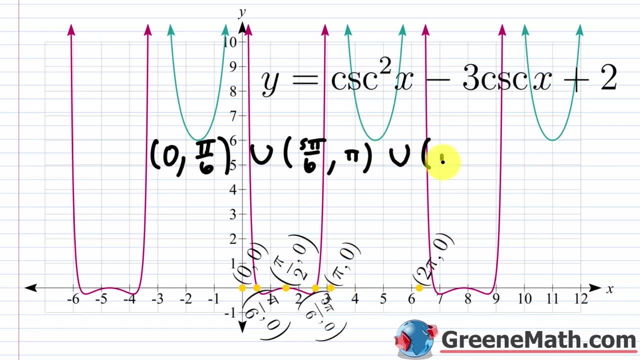 width, you would say: anything that's larger than pi. So anything that's larger than pi. well, this is going to work. again, you're going to be on this green graph right here And this is going to work up into the point to where you get to anything less than two pi. So again, that's. 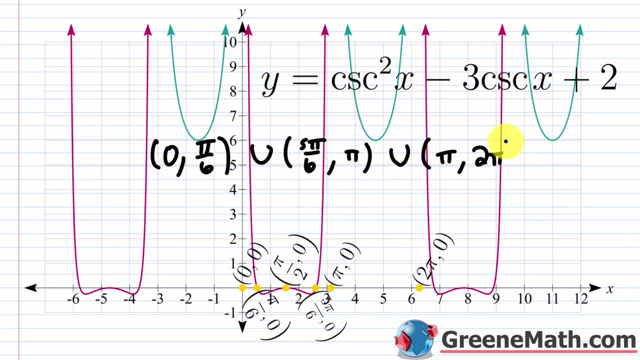 where you're undefined again. So from pi to two pi, with both being excluded. So if you want to go to Desmos and check this out, you can visually see our solution. So anything between zero and pi over six, and then also you could say anything between five, pi over six and pi, And then, lastly, 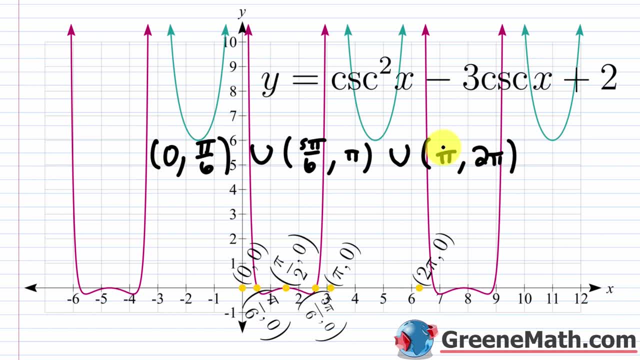 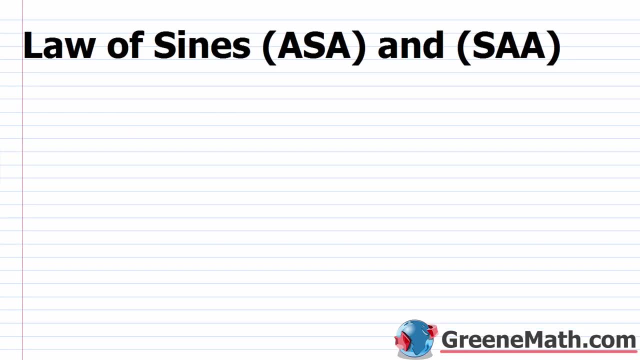 anything between pi and two pi. So all of those areas would work in the interval that we're solving over, which was from zero to two pi, with zero being included and two pi being excluded. In this lesson we want to talk about the law of sines And specifically here we'll look at the 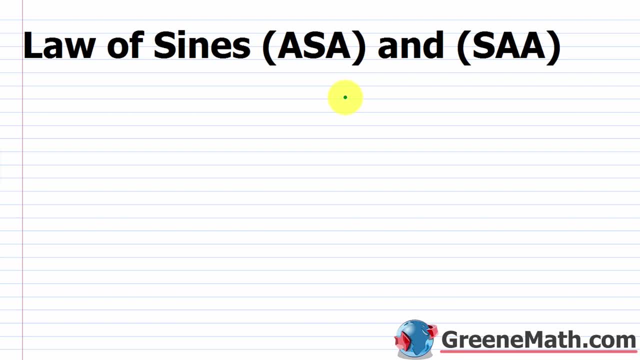 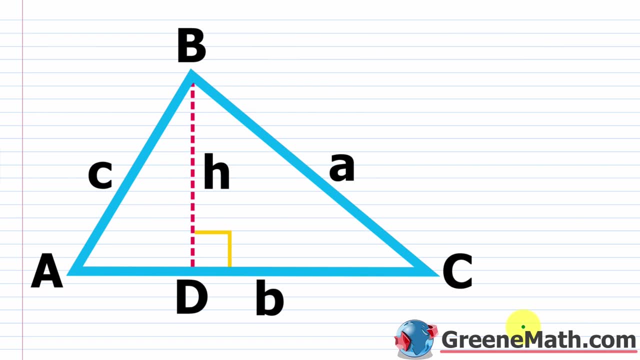 easier case where we have angle, side angle, And then also if we have the side angle angle, Okay. so before we jump in and look at problems, I want to talk a little bit about where the law of sines comes from, And so if you're not really interested in how this guy gets derived, you can just skip. 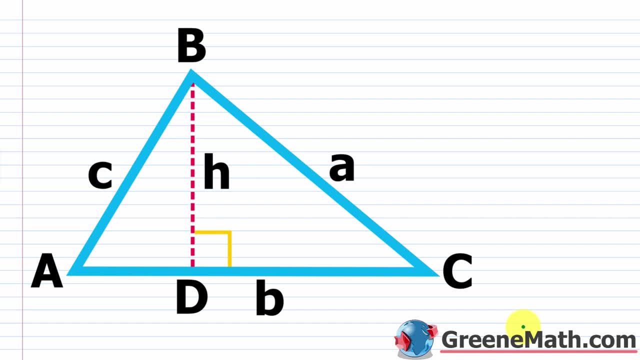 ahead to the examples. So the first thing is, when we talk about solving triangles- earlier in the lesson we talked about how to solve triangles with the SOHCAHTOA- right, This just means we're finding all the missing sides and all the missing angles. Now, when we work with an oblique triangle, 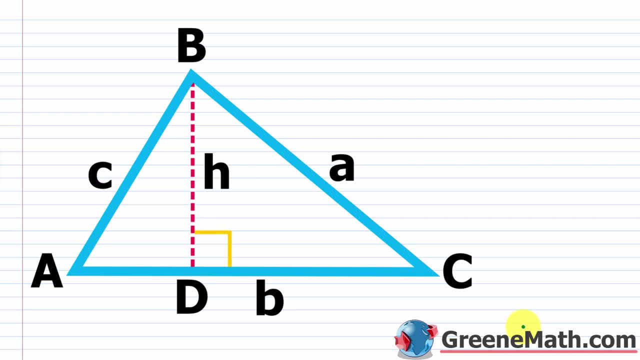 this is a non right triangle, then basically we have to use something like the law of sines or the law of cosines, because we don't have a right triangle, Okay, So basically, what I'm going to do is I'm going to start off with this acute triangle, okay, which? let's just go ahead and 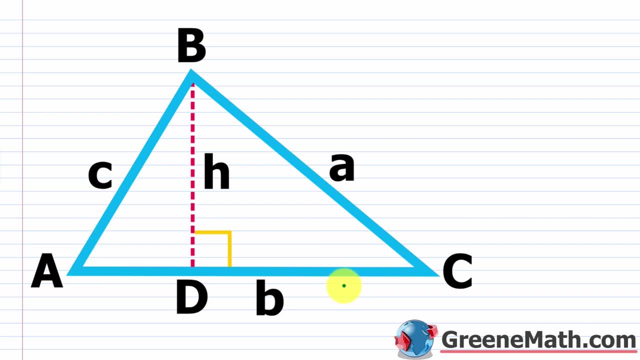 call it ABC, Okay. And I want to just draw your attention to a few things in terms of the naming conventions. So you see that you have capital letters, you have capital letters, you have capital letter A, capital letter B and capital letter C. those are your angles, okay, And then? 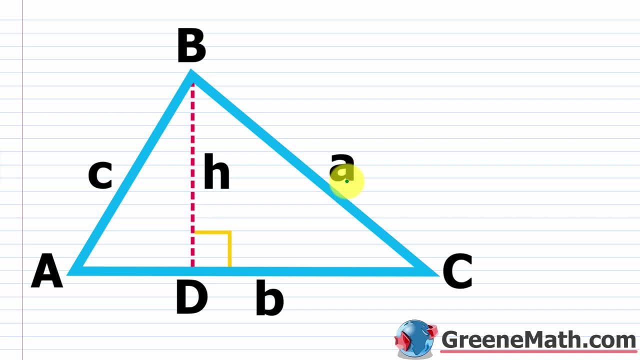 when you look at the lowercase letters, those are the sides, okay, that are across from their corresponding capital letter, angle, right? So what do I mean by that? In other words, this is angle A. if I go across, I have lowercase a. this is for the length of this side here. okay, That's all. 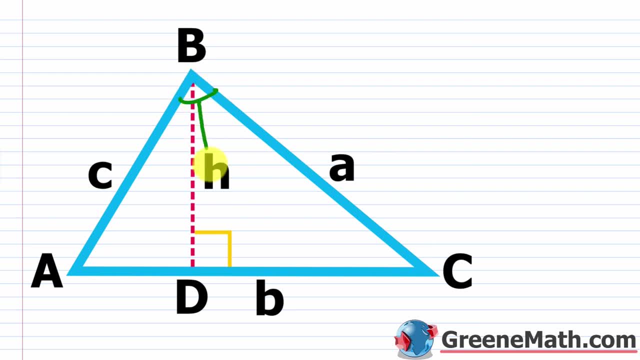 that is, If you look at B here. this angle right here, if I go across, this is B right, So it's the length of this side here, right. So on and so forth. you can do C as well. 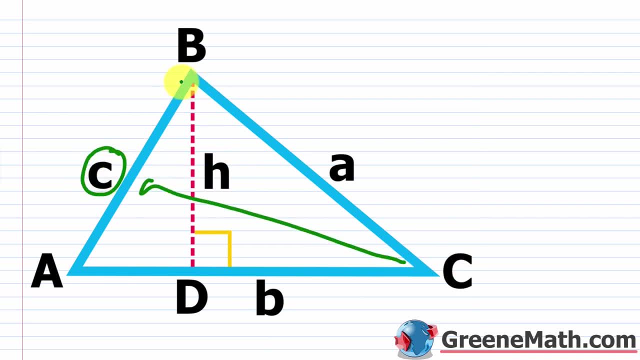 This is angle C, if I go across. okay, here's lowercase c here, so it's the length of this side. So you just need to understand how this is named, because pretty much in every book this is how they're going to do it. Now what I'm going to do, because we have an oblique triangle. 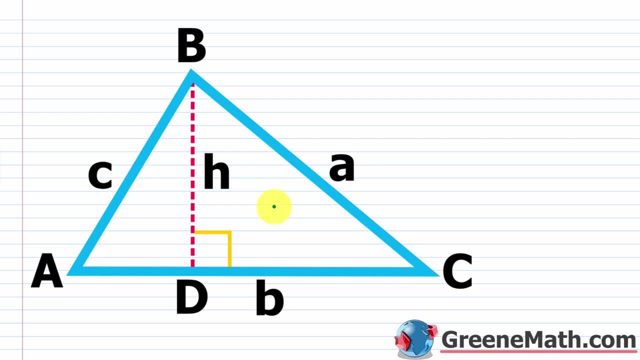 we're going to split this triangle ABC up into two different right triangles. okay, So you see, you have this perpendicular here that's been drawn and we've labeled this as H for the height. okay, You've seen this in geometry, where you basically have the height so you can get the. 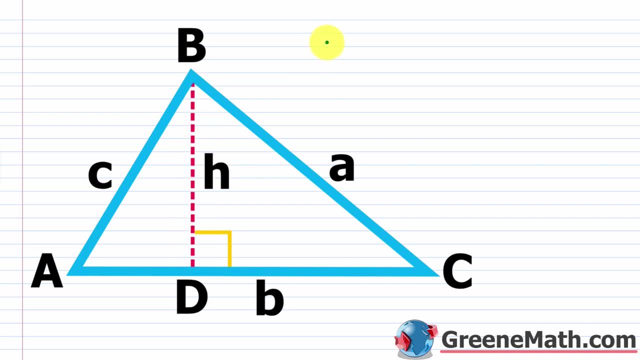 area, okay. So basically, what we would do here is think about the height of the triangle, these two separate triangles. So I'm going to say I have triangle triangle and I'll call the first one ADB, So ADB, okay. So if I think about that, that's ADB, like this, So that's a right. 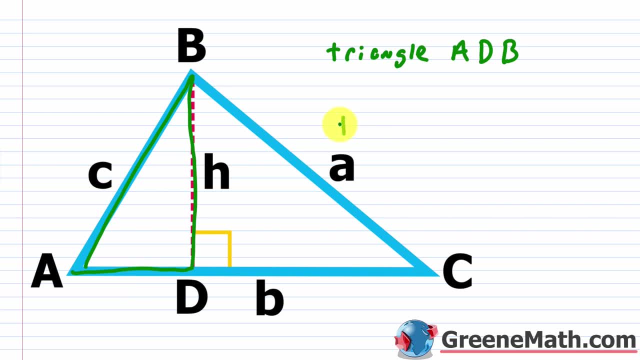 triangle, And then I also have another triangle that I'm going to form inside. So let's call this triangle okay, And let's go ahead and say this one's BDC. So let's say BDC, So BDC, like this: 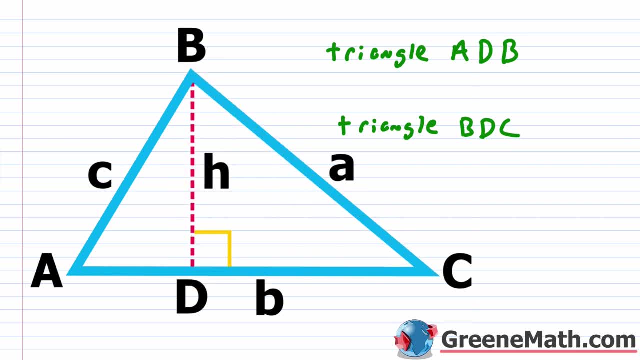 okay, So you see the two right triangles. Now let's think about, let's say, the sign of this angle here to start. So what is the sign of this angle? A Well, basically I'm going to think about the opposite here. 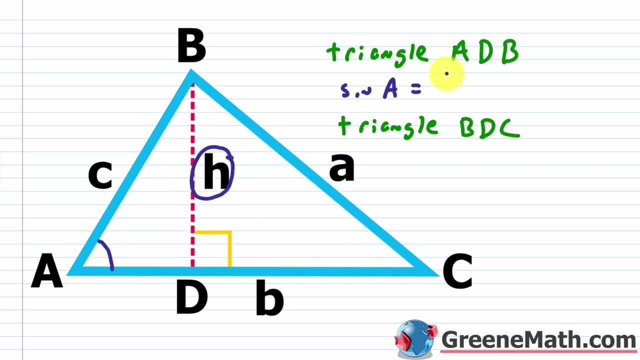 which, in this case, is H, right, If I'm thinking about this right triangle. So H over what's the hypotenuse? Well, in this case it's going to be C right. Again, you might have to highlight this. 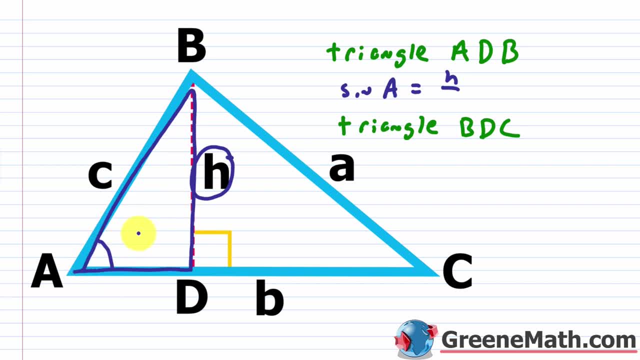 to really see. So this is ADB like this: If you think about this right triangle, this is your opposite and this is your hypotenuse. So this is H over C. okay, If you use a similar thought process. if you looked at C. okay, this angle here. 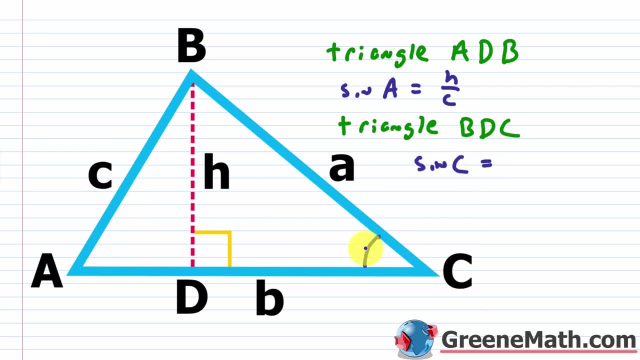 what is the sign of this C guy? Well, now it's going to be the opposite, which is H over the hypotenuse, which is A here. okay, So let's grab these two results and let's just write this over. 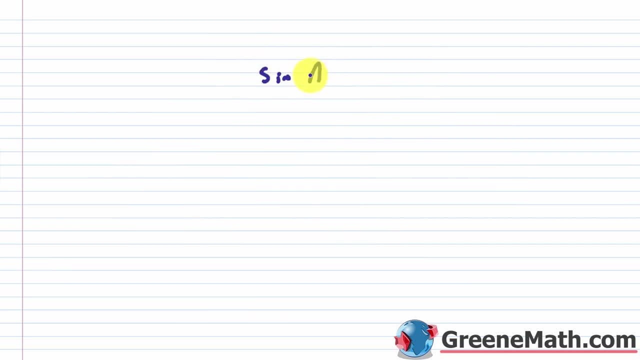 here. So I have the sign of this angle A here was H over C, And then I also have the sign of this angle C is H over A. okay, What you're going to do is you're going to write this over here. 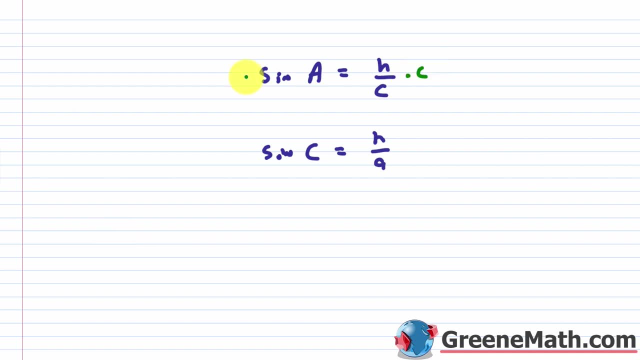 you're going to solve each one for H. So in other words, I would multiply this side by C and this side by C, And over here let me make sure this is lowercase so I don't confuse anybody Over here- this is going to be A and this is going to be A, So you multiply both sides here by A. 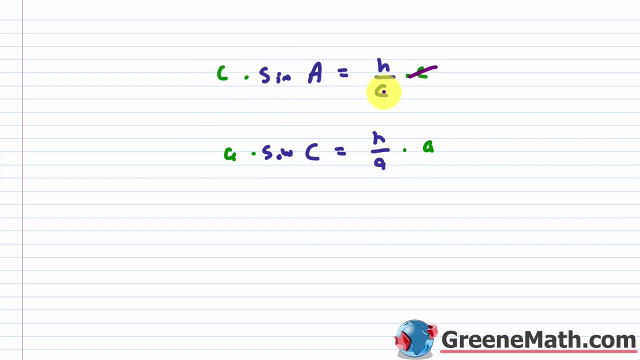 multiply both sides here by C. What's going to happen is this over here is going to cancel okay And this over here is going to cancel. So really I can just erase this and say that H here is equal to C times the sign of A, and H here is equal to A times the sign of C. 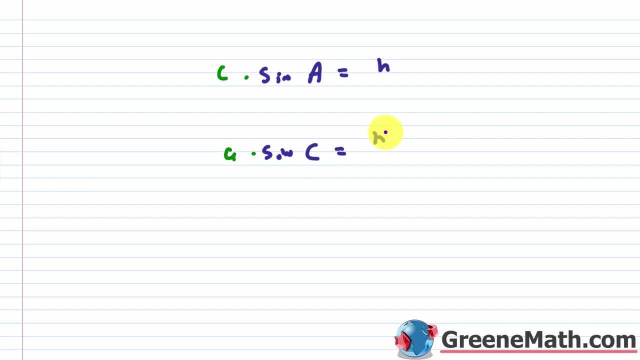 So since each one is set equal to H, I can set them equal to each other legally. So I can just erase this and I can just drag this up here, or actually I'll put this over here to match the convention in the book. So let me write this a little bit. 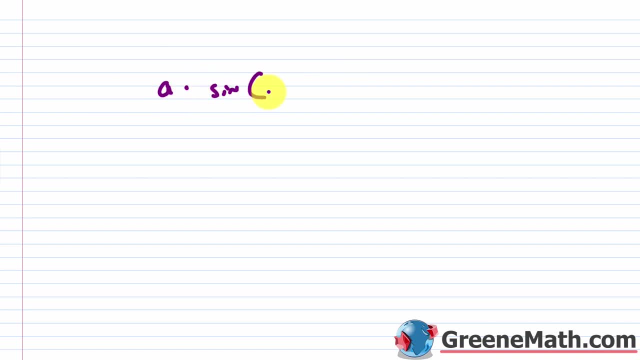 bigger. So A times the sign of C- okay- is equal to. you're going to have C times the sign of A, like this, okay. So what I want to do now is just divide both sides by the sign of A times the sign. 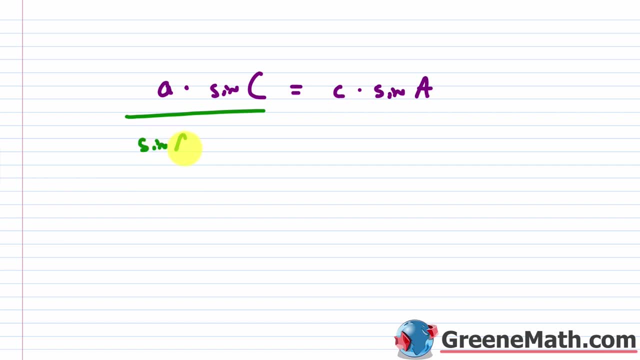 of C. So I'm going to divide this side by the sign of A times the sign of C- okay, And this side by the sign of C of A times the sign of C. So from here, I'm going to cancel this with this and I'm also going to 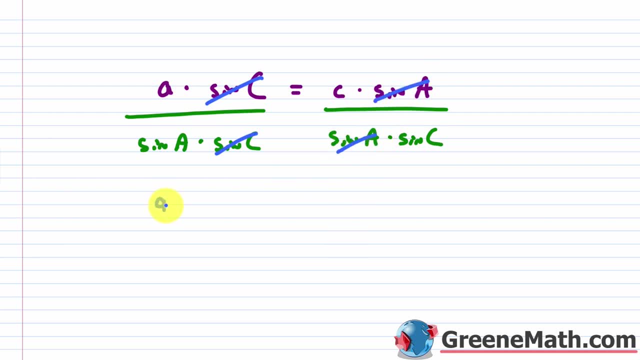 cancel this with this, And so what I get is I get this A over the sign of A. Let me make that better. So let me make that better. So sign of A like this is equal to the C. okay, The lowercase. 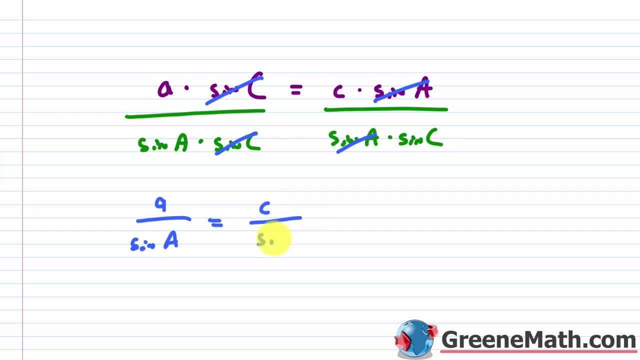 C is over the sign of C. okay, Like this. So what this is telling you is that, basically, the lengths of the sign of A times the sign of C is equal to the C times the sign of A. So what I'm going to 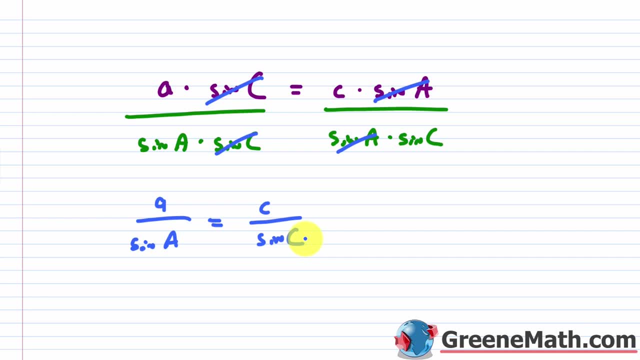 think about is that if I do the grad sheets hiding in this example and pick one side and this little dot and move the corner while I'm working on here- you can look at my experiments here- Make sure you're creating these чет suites. 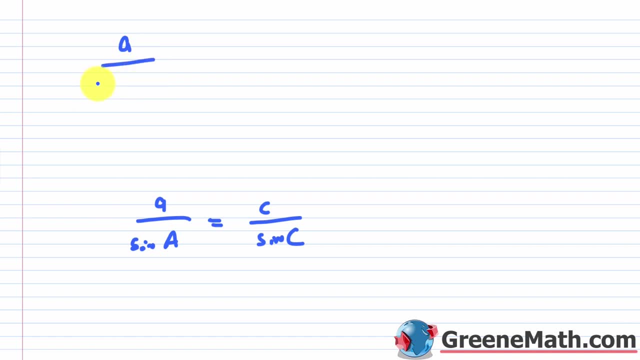 So two sides on A times the sign of C. Two sides in the triangle are proportional to the signs of the measures of the angles opposite them. We could also do a similar process to show that C, so I could also put C over the sine of C. okay, so you can go through and prove that to yourself. 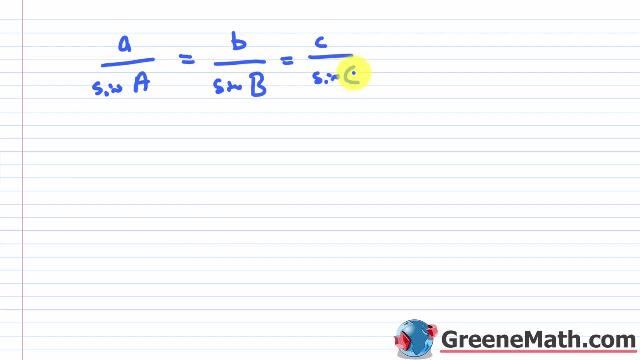 if you want to go back to the triangle, but this is basically what we're going to be using throughout this lesson. it's very, very easy. okay, overall, you're just going to use one part, so, in other words, you'll either use this guy right here, or you'll use this guy right here, or you'll use the. 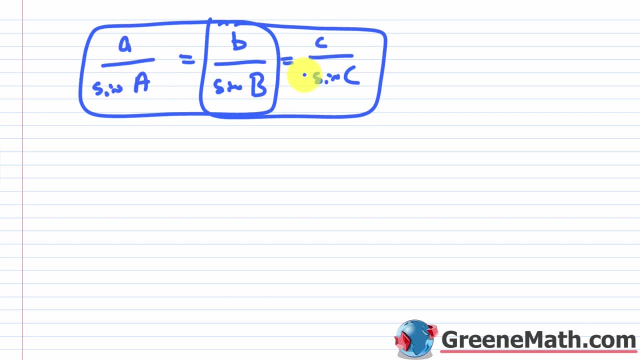 original one we had, which is A over the sine of A is equal to C over the sine of C. okay, so let's go ahead and jump in and look at an example. so we're given that B, which, again, if you get a capital letter, this is an angle- is equal to 46 degrees, C is equal to 69 degrees and A is 34 centimeters. 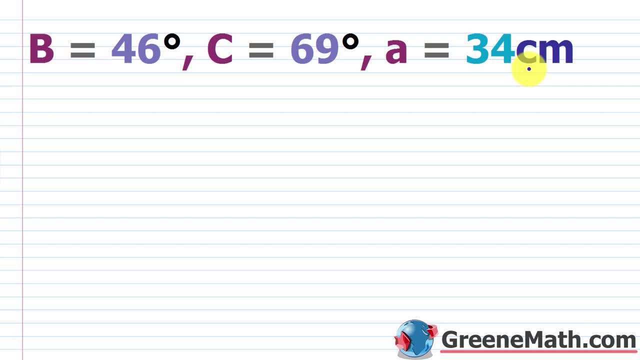 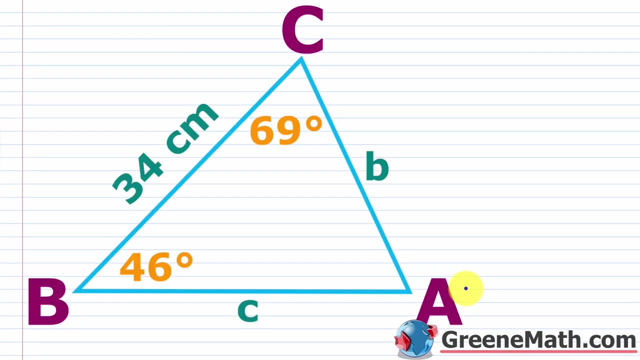 so I'm going to tell you, like most people will, when you start these problems, just make sure you draw a little sketch. it doesn't matter if it's accurate at all, you just want something to put numbers down, all right. so I've already pre-drawn this little sketch for us. so you see that your 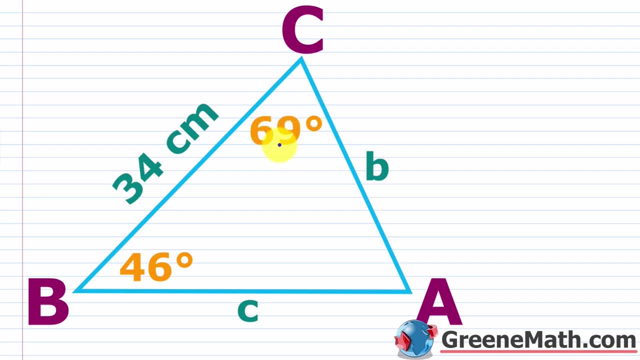 angle B here is 46 degrees, your angle C here is 69 degrees. and then this guy, if you go opposite of A, you're going to get a little bit of A, and then you're going to get a little bit of B, and then this is your A. here it's 34 centimeters. okay, so now, if I think about what I need to find, I need: 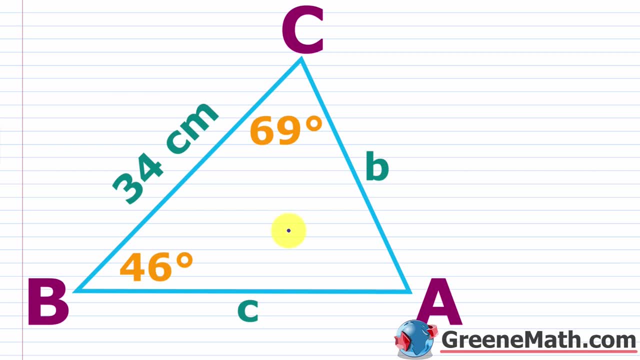 to find the measure of angle A. so let's go ahead and do that. first, remember: your triangle sum property tells you that the angles inside of a triangle are going to sum to 180 degrees. so on a calculator you could go 180 degrees minus 69 degrees minus 46 degrees and this is going to 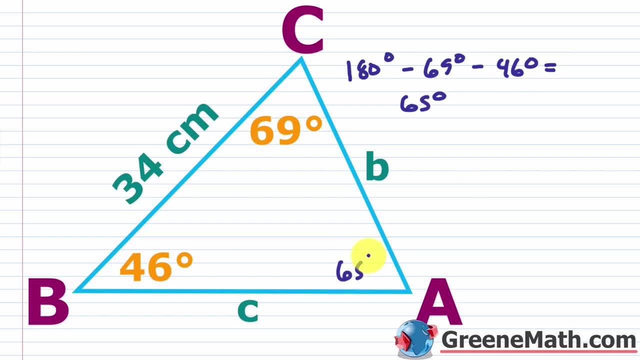 give you 65 degrees. okay, so you can go ahead and put a 65 degrees in there, like that. okay, so that's going to give you that 65 degrees. and then I'm going to draw this out and some will say: okay, I want your answer. so we'll say: a is equal to 65 degrees here, like that. so we'll do both, okay in. 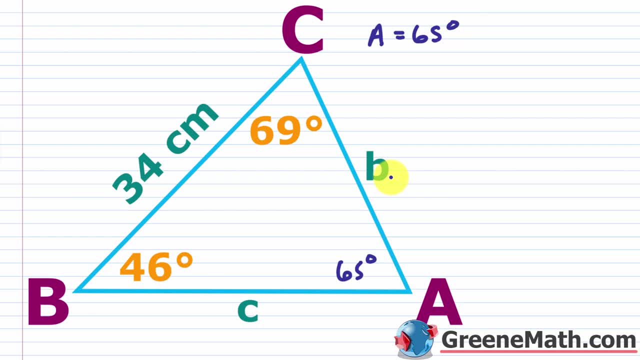 terms of B. how are we going to figure this out? we've got to work with what you have. so, in other words, I have an angle measure a and I have lowercase a, the side length. okay, so I can say that a over the sine of a is equal to B over the sine of B. okay, so I can just plug in for a here. 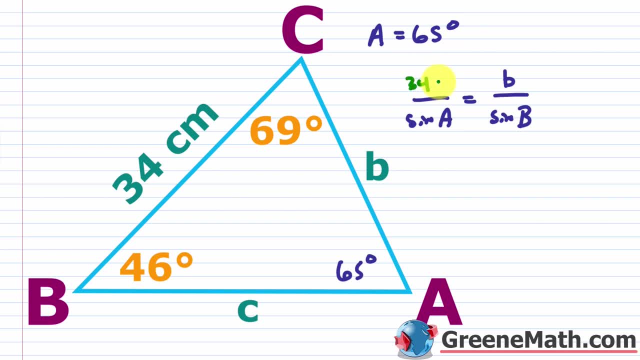 34 centimeters. So this is 34 centimeters. And then for the sine of A, you're taking the sine of 65 degrees. So the sine of 65 degrees, Then for this guy right here, B over the sine of B. 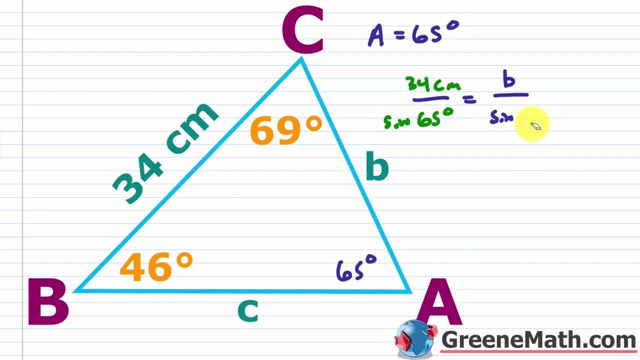 well, B, the capital letter B, is 46 degrees. So we're going to put 46 degrees there And basically, if you want to solve this guy for B, right lowercase B, you would say that lowercase B is equal to. you're just going to multiply both sides by the sine of 46 degrees. 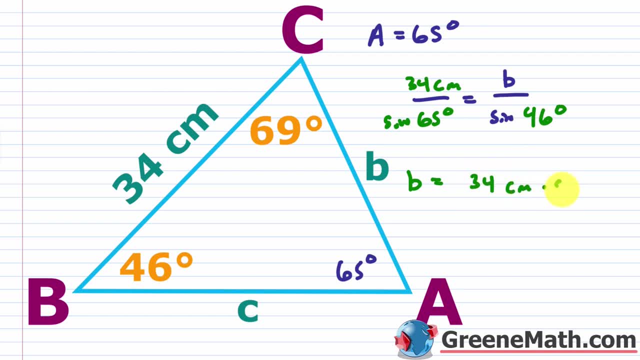 So you would say 34 centimeters times the sine of 46 degrees over the sine of 65 degrees. Now if I punch that up on my calculator, I get about 26.9859.. Okay, Let's just go ahead and round this. 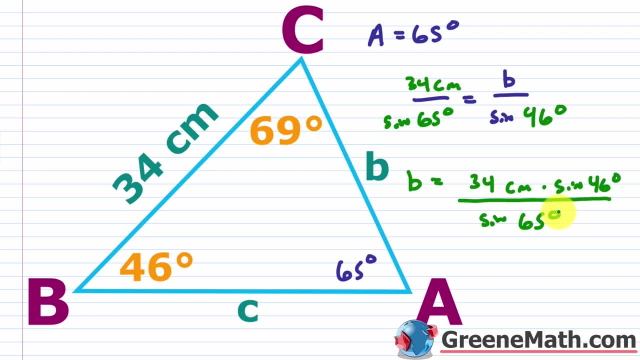 to the nearest 10th. Okay, So I'm going to say that would be about 27.. So let's just approximate this. I'm just going to erase all this And I'm going to use the approximately symbol. Okay So. 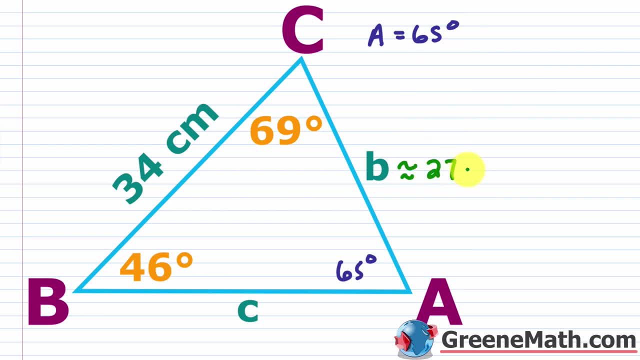 I'm going to put approximately Approximately 27.. Okay, And this should be in terms of centimeters, So let's put this up here. So B is approximately 27 centimeters, And in terms of where you need a round, just get with. 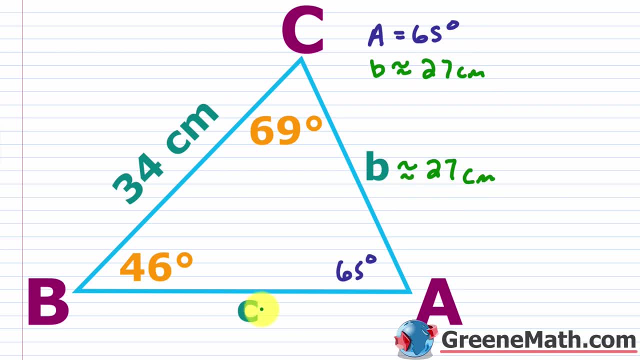 your teacher or your assignment. It should tell you Now for C. the mistake that a lot of people make is they use this rounded value. You want to stick with the information you're given. You're given a hard coded value here of 34 centimeters. Just use that again. So I'm going to want to do. 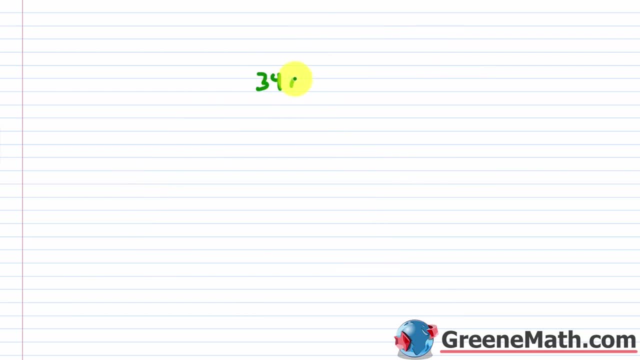 let me do this on another page. I'll do A, which is 34 centimeters Over the sine, Okay, Of A, Let me make that better. So the sine of A, which was, again it's 65 degrees, is equal to. you're going to have lowercase C over the sine of what was our angle C. 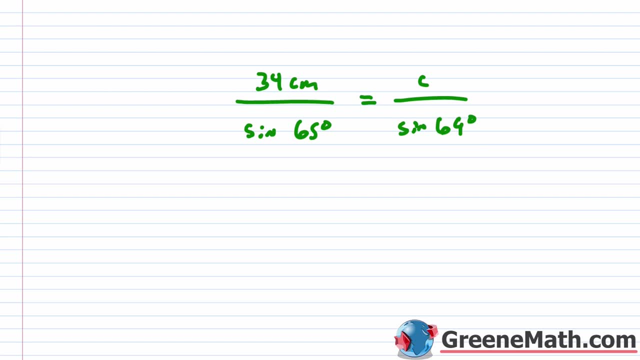 that was 69 degrees, Okay. So again, very easy to do overall. You're just going to multiply both sides by sine of 69 degrees, So you're going to have 34 centimeters times the sine of 69 degrees. Okay, Over the sine. 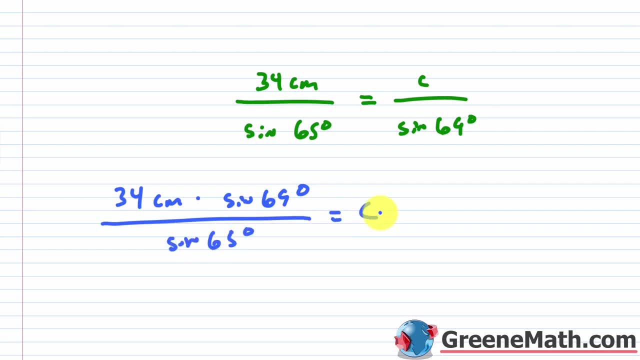 Of 65 degrees. Okay, So this is what C is going to be. So let's erase this. So this would give me about 35.023.. Let's say one Again. if you want to go to the nearest 10th, we'll just say 35.. 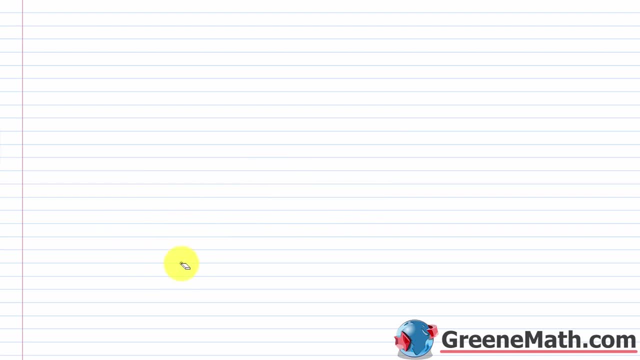 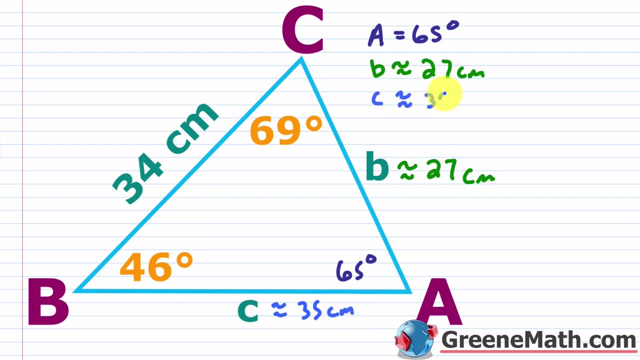 So let's just erase this, We don't need it anymore. And we'll go back up and we'll say that this is about 35 centimeters. So you can put this here: C is about 35 centimeters. So just depending on what your teacher asks for, you might want to list things like this: 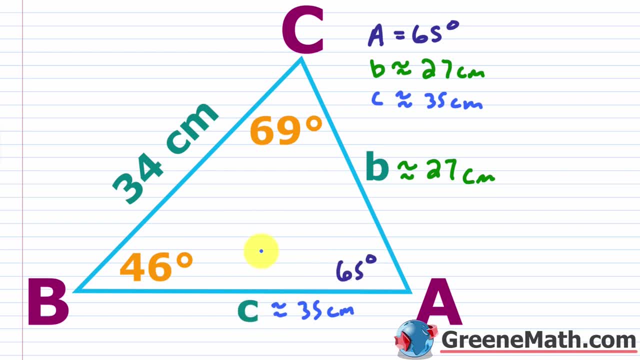 you might be asked to draw a triangle and then fill in the missing parts. whatever it is, just make sure you have all the missing sides. Okay, Here we got. B is about 27 centimeters, C is about 35 centimeters, And then you're missing angle, which here is 65 degrees. Okay, Let's look. 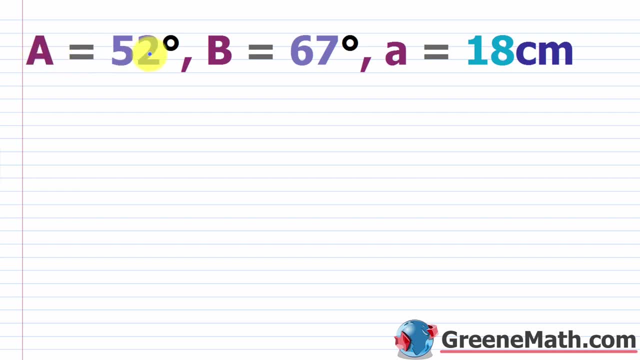 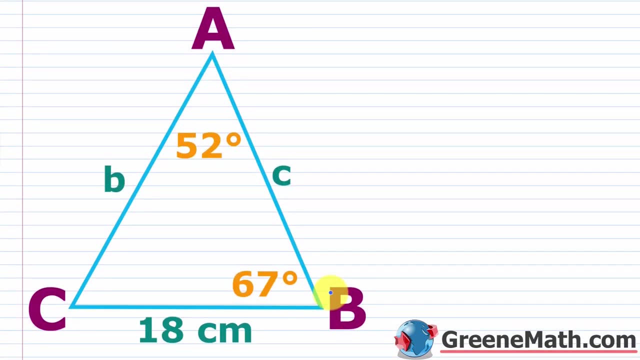 at another one. Again, these are very, very easy. So A here is 52 degrees, B here is 67 degrees, and A lowercase A is 18 centimeters, So let's go down. And so again, A is 52 degrees, B is 67. 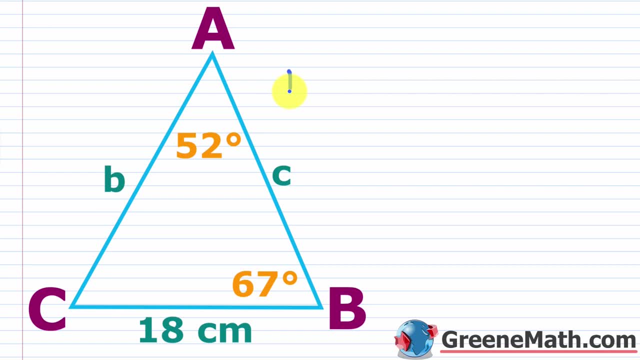 and basically C is unknown, But again, we can find that really quickly. Just go ahead and do 180 degrees minus 52 degrees, minus 67 degrees And that's going to give you 61 degrees. Okay, So let's put that in there. So this is 61 degrees And again, you might want to list this up here. 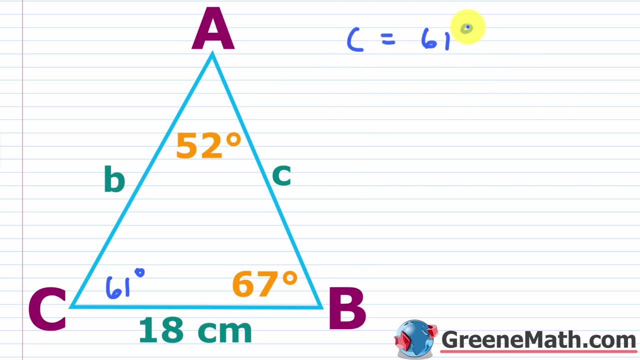 So let's say C is equal to 61 degrees, And then we want to find B and C here. Okay, So I have my angle measure 52 degrees here for angle A, and then side A is 18 centimeters. So again, I can just set. 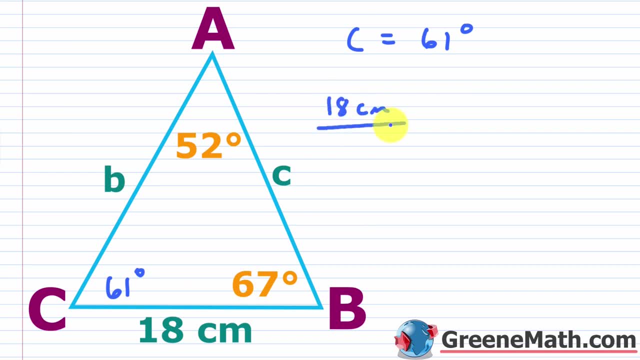 this up, I can say 18 centimeters. 18 centimeters over the sine of this angle A, which is 52 degrees, is equal to- let's just go ahead and start with B, So I'll say B over the sine of 67 degrees. Okay, And if you? 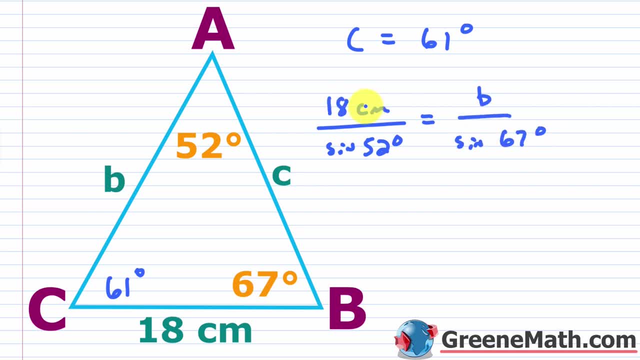 haven't noticed. basically this guy right here always ends up being multiplied by this, So a shorter way to do this would be: B is equal to. you know, basically the sine of whatever this angle is: times this ratio here. Okay, That's all you need to do. So let's go ahead and say B. 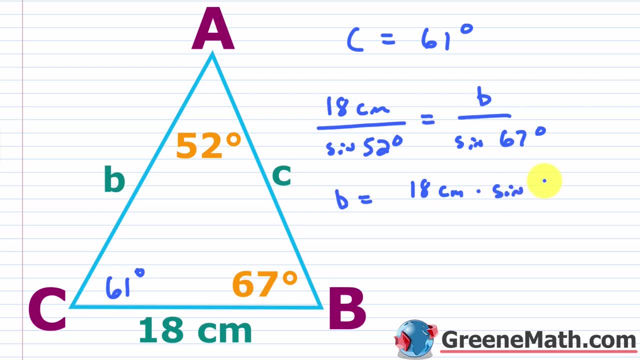 is equal to 18 centimeters times the sine of 67 degrees over the sine of 52 degrees. Let me just erase this, So I get about 21.026, let's say five. Okay, And let's round this to the nearest 10th. 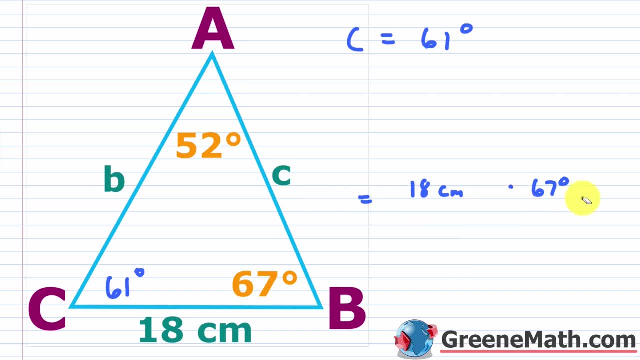 So that's going to give us about 21.. So let me erase this and I'll say that this is about approximately 21.. And don't forget your units. So we'll say, okay, B is approximately. okay, Approximately 21 centimeters. Okay For C, let's use a little. 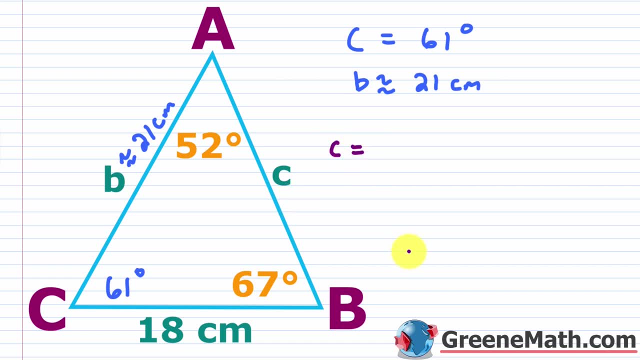 shortcut. Okay, Let's go ahead and say that C is equal to. again, I want this guy right here, 18 centimeters. Okay, Over this angle, here, the sine of this guy, So the sine of 52 degrees. 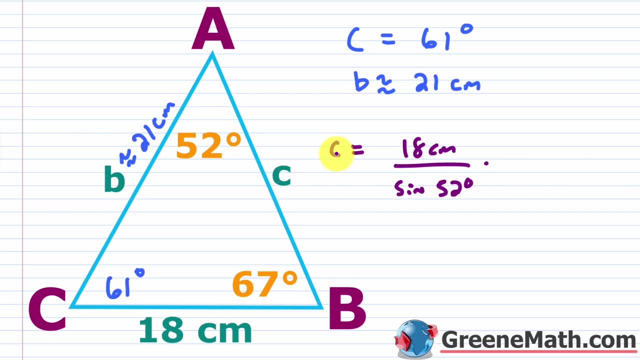 but I'm multiplying this by again. remember, you would have had C over the sine of C, which is the sine of 61 degrees. but we multiply both by that guy. Okay, So we can clear it. So this is times the sine of this angle here. 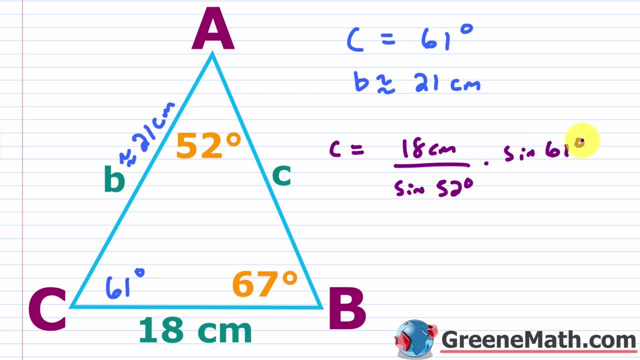 which is 61 degrees. Okay, No need to do two steps when you can do it in one. So if we go ahead and crank this out, you're going to get about 19.9784.. Let's go ahead and round this to the nearest 10th. Let's just say it's about 20.. Okay, So 20 centimeters. So let's. 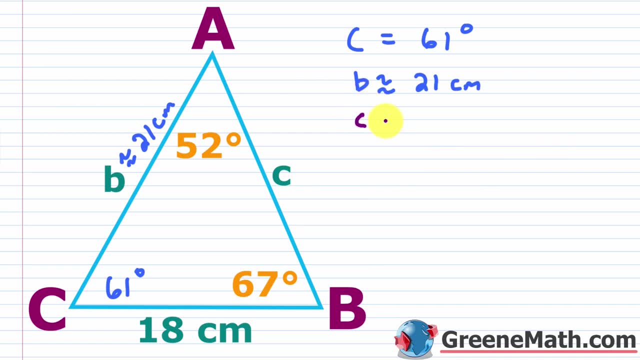 erase this and I'll say lowercase: C here is approximately 20 centimeters And again, you can write it in here if you want to. So 20 centimeters, Okay. So we found C is about 20 centimeters, B is about 21 centimeters and angle: 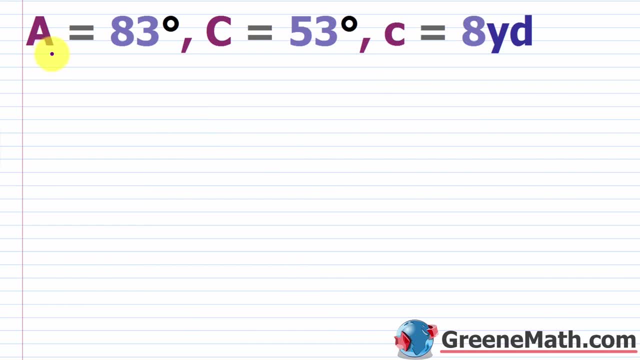 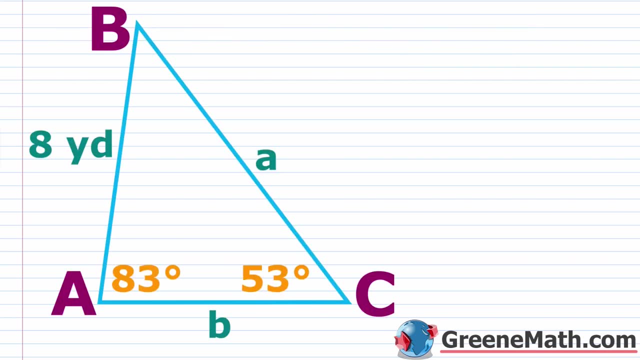 C: here is 61 degrees. Let's just look at one more. So we have: A is equal to 83 degrees, C is equal to 53 degrees and lowercase C: here the side length is eight yards. Again, we have our lowercase A. 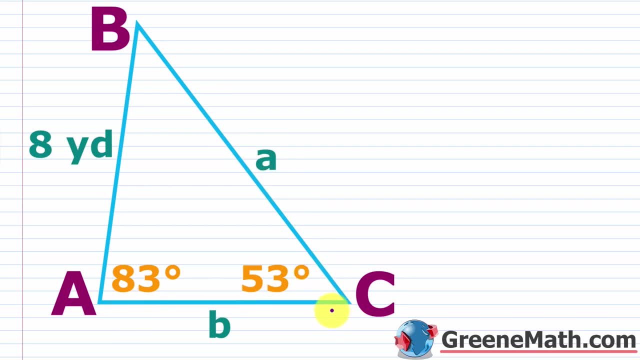 this side here we need to solve for lowercase B. this side we need to solve for, And we don't know the measure of this angle B. I always start with the measure of the angle because it's the easiest. So you want 180 degrees minus 80.. 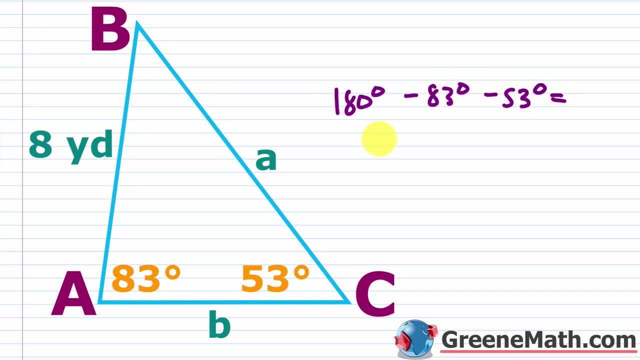 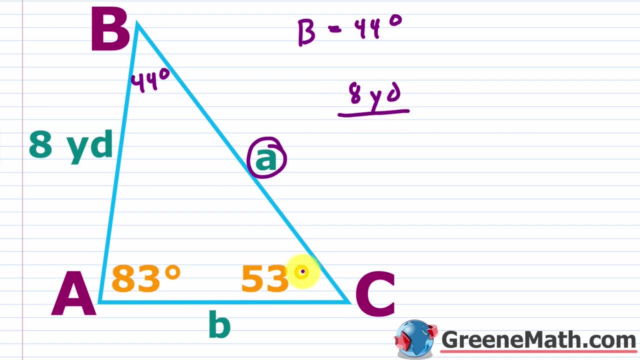 where I say eight yards, okay, over, let's go ahead and say the sign of 53 degrees, Okay. So if I wanted A, so A would be equal to what It would be this times the sign of this angle here, Okay. 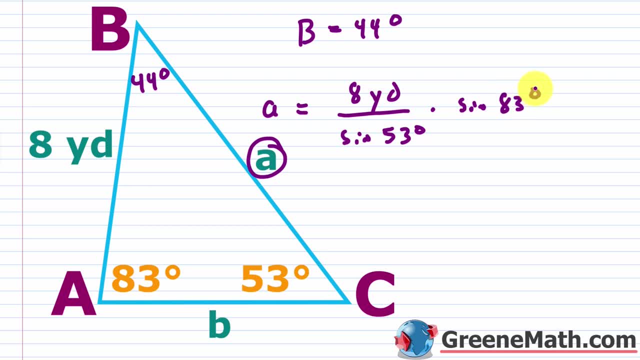 So the sign of this 83 degrees. Okay, So you set that one up and then for B, B would be equal to. again, I'm going to keep this part the same. So eight yards over the sign of 53 degrees. 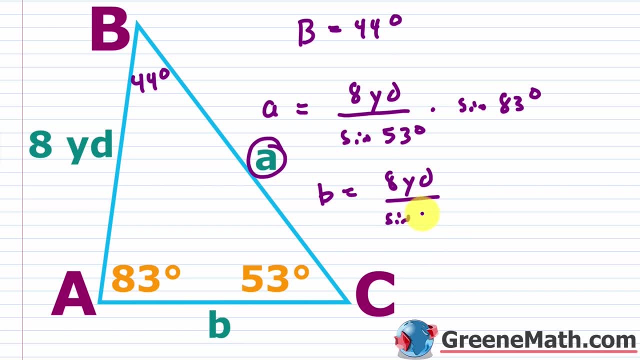 Let me make this better. So sine of 53 degrees and then times the sine now of: in this case, the angle b is going to be 44 degrees. okay, so 44 degrees there, all right. so let's start with a. let's punch that up on our calculator. so 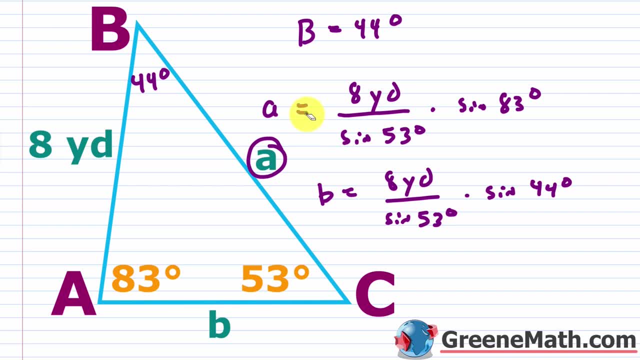 if i round this to the nearest tenth, i'll just go ahead and say it's about 9.9, so 9.9 and this is yards, so i'll say approximately. let's answer it twice. so here i'll put approximately 9.9 yards. 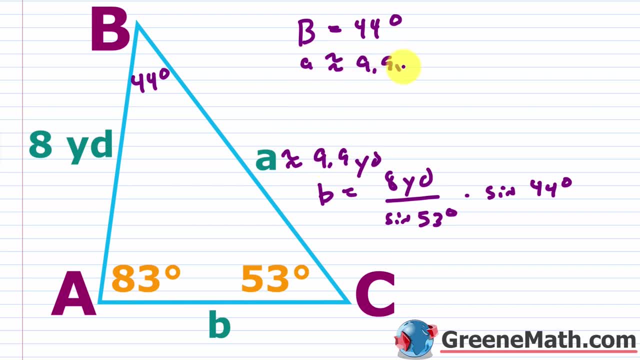 and i'll do it up here as well. so a is approximately 9.9 yards, and then, for this one, let's just go ahead and say that's about seven. right again, rounding to the nearest tenth, so it's about seven. so let me get rid of this and i'll say this is approximately seven yards, and then up here, 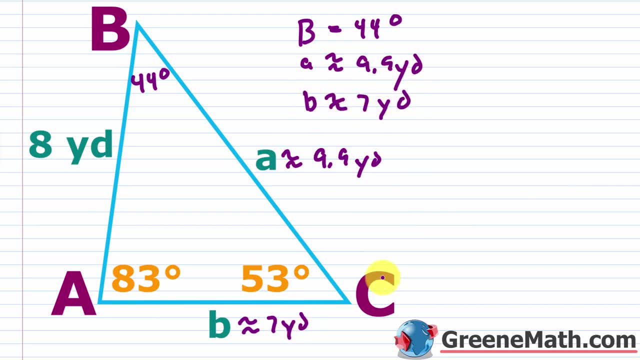 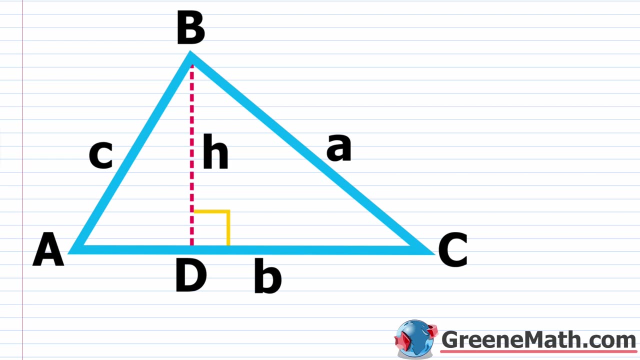 b is approximately seven yards. okay, so again we found that a is about 9.9 yards, b is about seven yards, and then this missing angle measure of capital letter b here is 44 degrees. okay, so another thing you're going to see in this section is about the area of a triangle, so this is going to involve side angle. 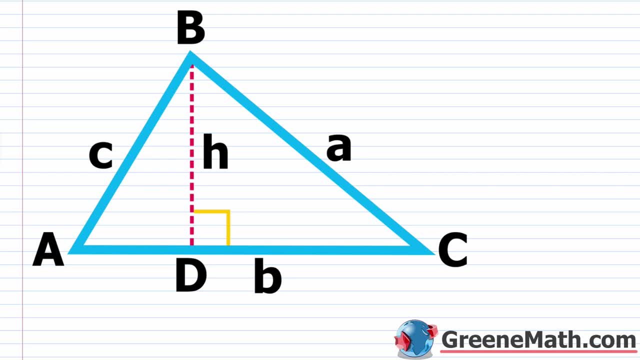 sides, so you're going to have two sides, okay, and the angle between them. so the method used to derive the law of sines can also be used to derive a little formula to find the area of a triangle. so i want you to recall from basic geometry, the area is equal to one half times the base. 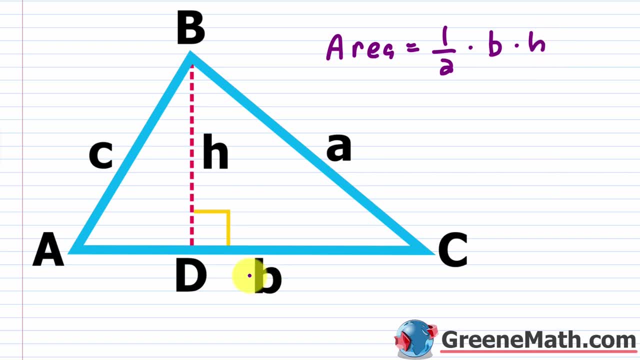 times the height. okay, so here our base would be this lowercase b, right, because that's this side here right, and then our height would be this h here- okay, this guy right here, and then our היה. so basically, i want you to think about our right triangle adb again, again, if we did sine of a, so 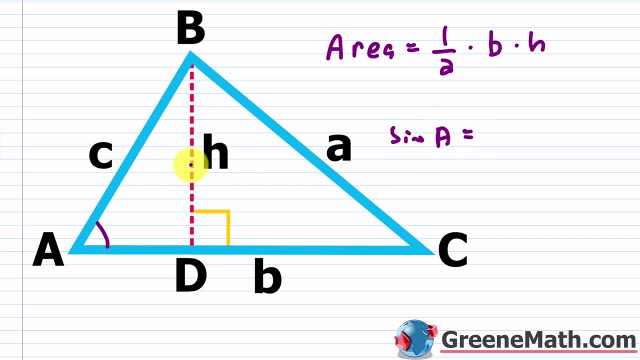 sine of a. this is equal to, again, h over c, so h over c. now, if i solve this for h, i'm going to. i'm going to get: sine of a times c is equal to h. so sine of a, sine of a times c, is equal to h. so i'm going to plug this in right here into this formula. okay, so i'm plugging this in. 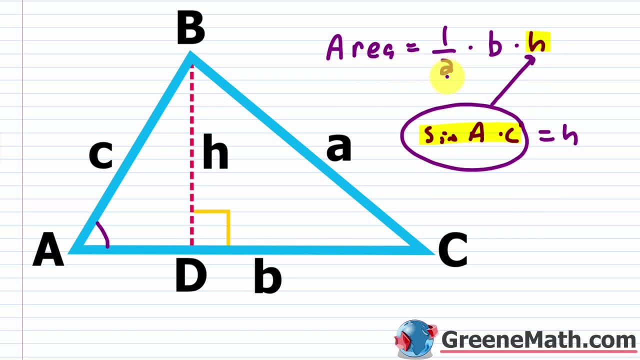 right there. so what i'm going to get is that this is going to be the varies that i'm going to get. the area is equal to one half times the base times. instead of H, I'm going to have basically C times the sine of A, So let's erase this and put C times the sine of A. okay Now, similarly, 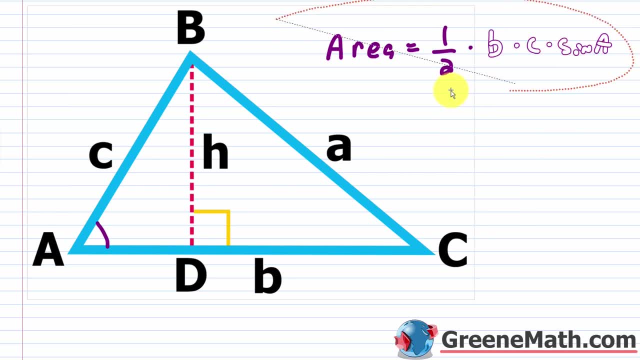 you could go through and calculate other formulas, okay, using a similar thought process. So you could say: the area is equal to one half times this. now let's go A times B. okay, then times the sine of C, and then, lastly, let's go: area is equal to one half times. let's see what. 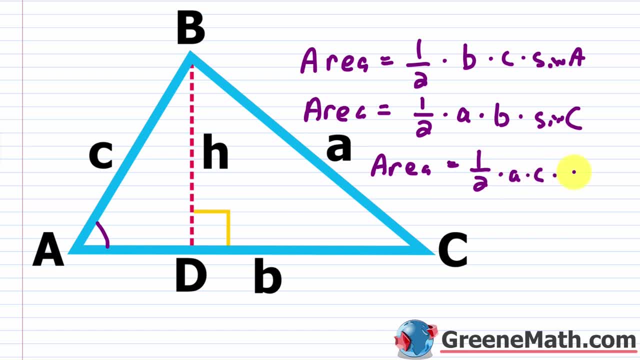 didn't we use. So it's going to be A times C and then times the sine of B, okay, So notice that this capital letter that's involved. okay, this angle is always the one that's not involved here, I know. 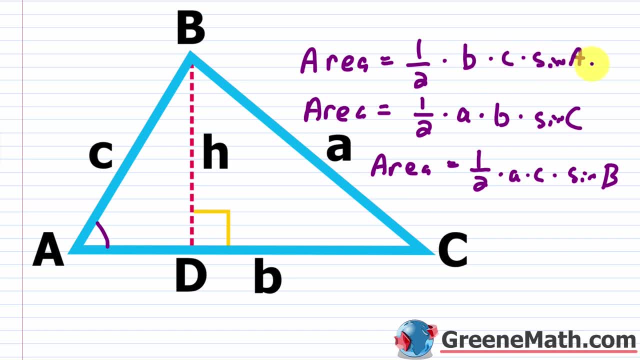 these are lowercase, but if you look, you have lowercase b and lowercase c. this is uppercase A, Lowercase a, lowercase b, uppercase c. Lowercase a, lowercase c, uppercase b. okay, And that's because you have lowercase a, lowercase b, uppercase c and lowercase c, uppercase b. okay. 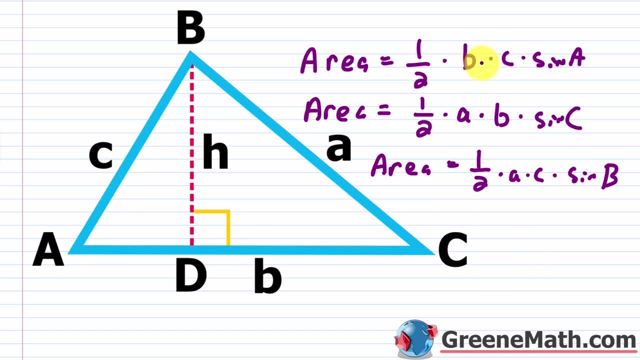 Because if you look at the way this is set up, if you have side B and side C, so this is side B and this is side C, so where's the angle between them? Well, that's going to be this guy right here. 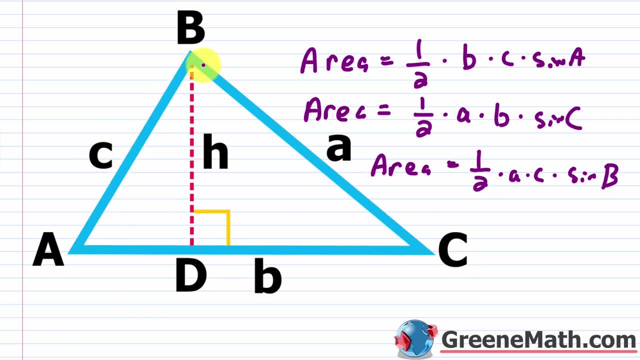 it's going to be A right. If I looked at A and B, so those sides. so this is side A and this is side B. okay, what's the angle between them? It's going to be C If I look at the last. 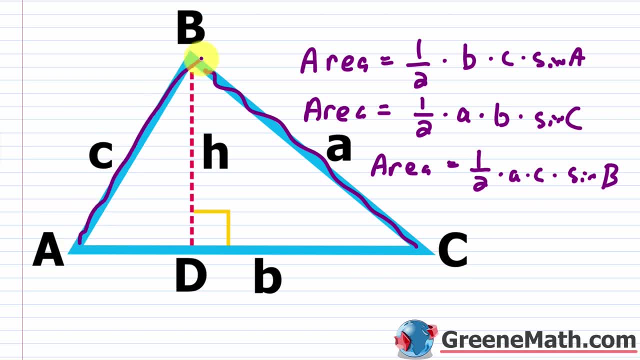 one which is A and C. so if I look at A and I look at C, what's the angle between them? It's going to be B, okay. So this is a little formula you can use, okay, because in some cases you're. 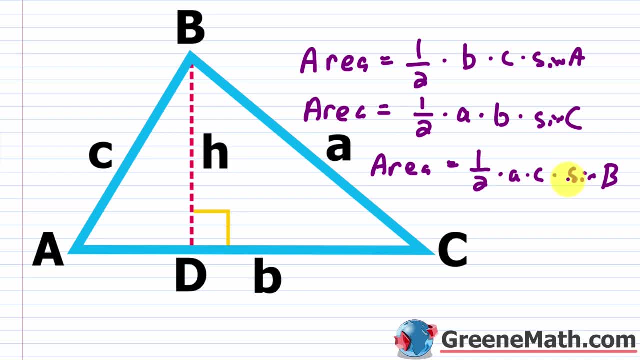 not going to know the height, you're not going to know what H is. okay, So you can basically use this instead. All right, let's look at this example here. So B here is 5 kilometers, A here is 10. 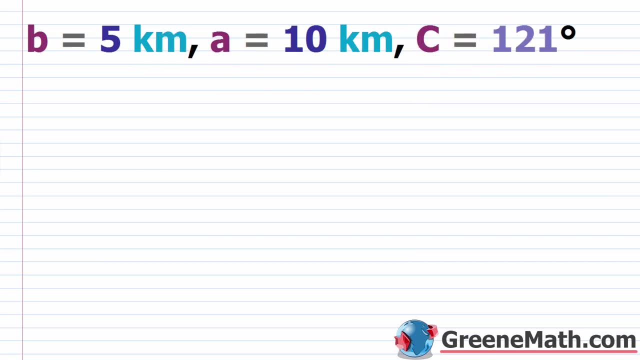 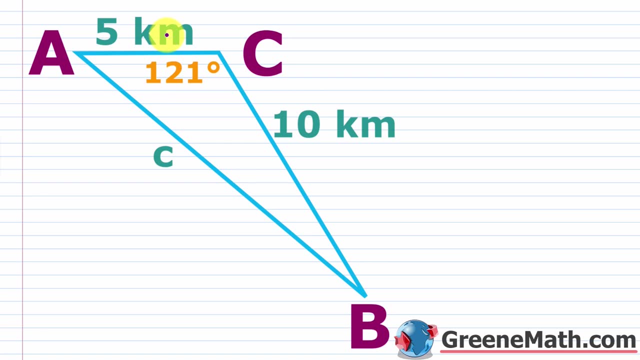 kilometers and C here is 121 degrees. okay, So again you sketch yourself a little diagram and basically we have again the side B here is going to be 5 kilometers. If I look at the side A here it's 10 kilometers and we know that C is 121 degrees. So again you have this side here. 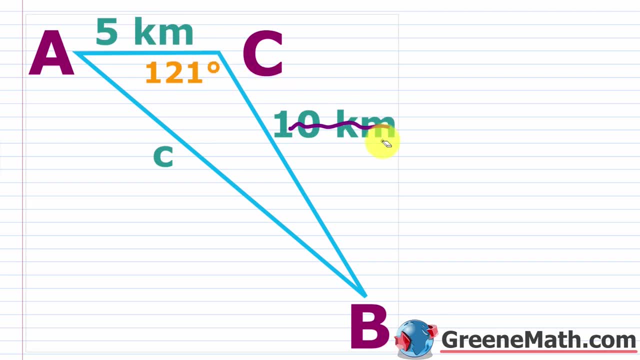 you have this angle, you have this side. here Again, notice that the angle is between them. okay, It's very important. So how do we do this? Well, again, we'll say the area. the area is equal to. I'm going to go one half times again. you take these sides, so 5 kilometers. 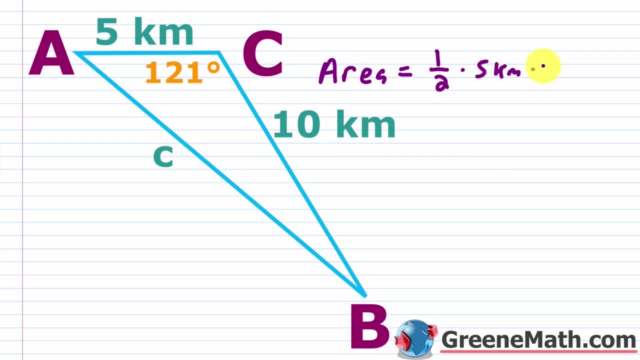 so 5 kilometers, times you're going to go 10 kilometers. so 10 kilometers and then times- let me kind of, this is going to run off the screen, so let me drag this over a little bit- so then times the sine of the angle between them, so the sine of 121 degrees, okay. 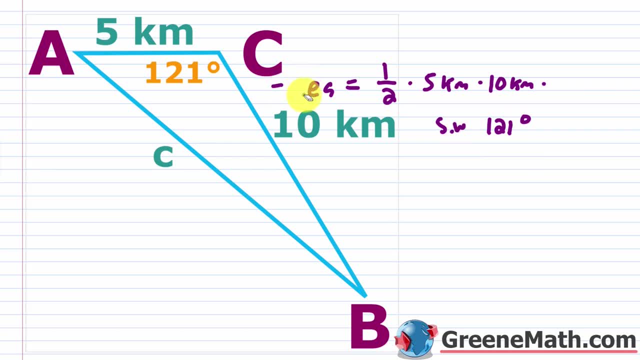 And so let's just go ahead and crank this out and actually, since it doesn't fit on the screen very well, let me kind of simplify this here. So 5 times 10 is 50,. 50 divided by 2 is 25,. 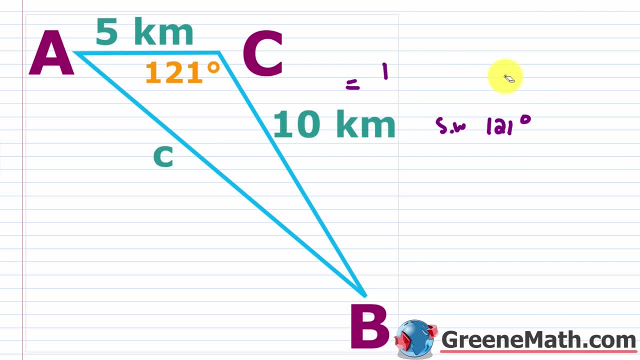 kilometers times kilometers is going to be kilometers squared. So let me get rid of all of this and say that the area, the area, is going to be 25 kilometers squared, okay, And then basically times the sine of 121 degrees. So let's just go ahead and punch this up into our calculator. 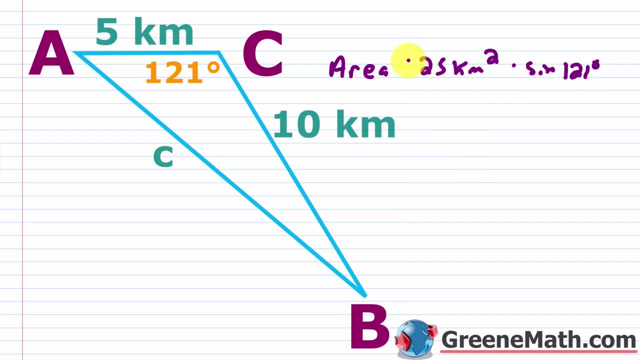 just do 25.. 25 times the sine of 121 degrees, and I'll go ahead and say that it's about 21.4.. Again, if you're rounding to the nearest 10th, so the area is about, okay, approximately 21.4,. 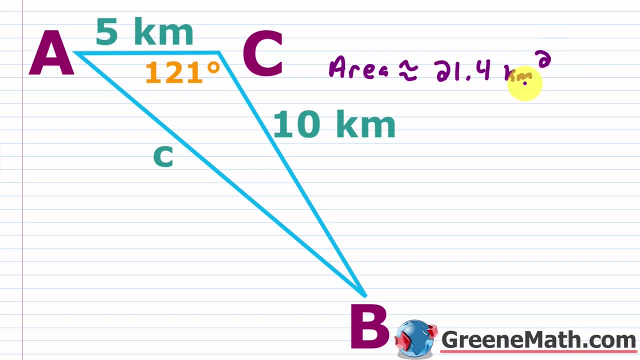 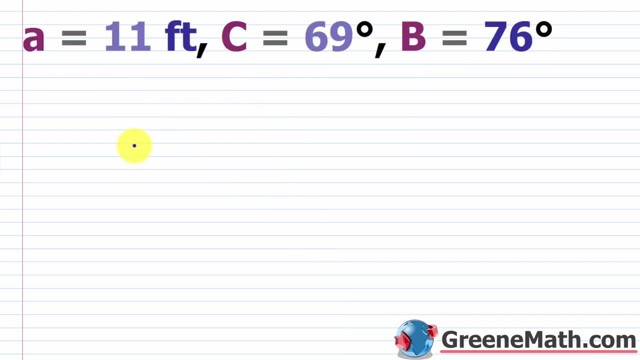 and it's going to be kilometers again. this is squared. Very important that you square your units there, because again you end up multiplying the kilometers times the kilometers, so you get kilometers squared. Okay, let me throw a wrench at you, So this is kind of a harder problem. 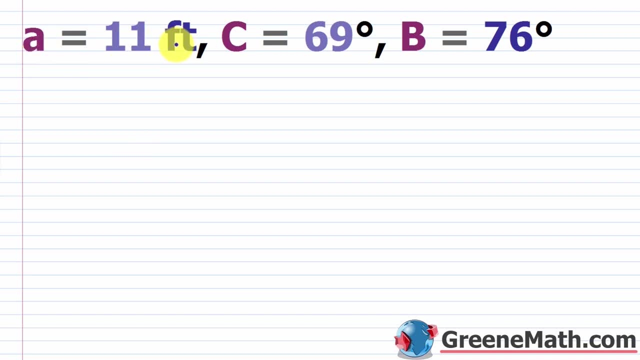 a harder variation of this problem. So you have: A is 11 feet, C is 69 degrees and B is 11.5.. So you have: A is 11 feet, C is 69 degrees and B is 11.5.. So you have: A is 11 feet. 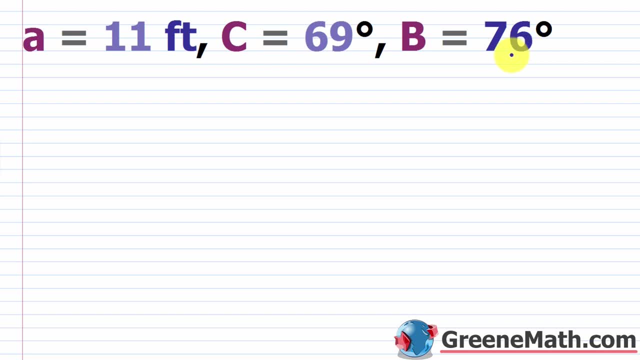 and B is 76 degrees. So you've seen the pattern before with side angle, side right where the angle is between them. But this one you have two angles and a side. So if I go down to my little sketch here, you see you have these two angles and this side here. okay, So basically to solve. 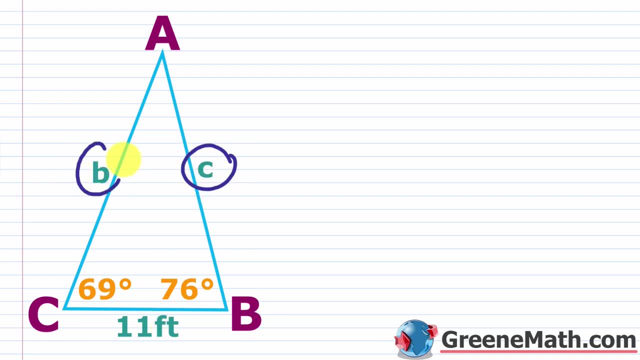 this guy to find the area. I either need to figure out C or I need to figure out B. okay, It doesn't matter which one you do, you're going to get the same answer. But basically, if I had C, 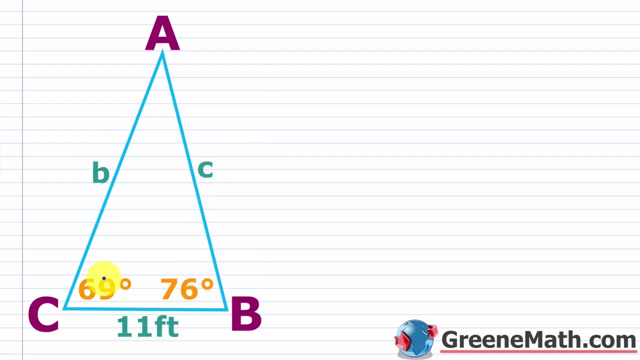 you have a side, an angle and a side. If you had B, you'd have a side, an angle and a side, So let's just go ahead and do B, okay? So we're given this 11 feet here. So to use the law of sines, I've got to first work with A, find the angle measure. 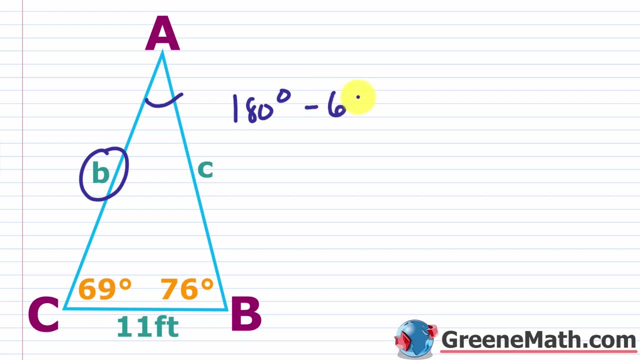 here. So that's going to be 180 degrees minus 69 degrees, minus 76 degrees, which is what? Well, that's going to be 35 degrees. okay, So this right here is going to be 35 degrees, So let's erase. 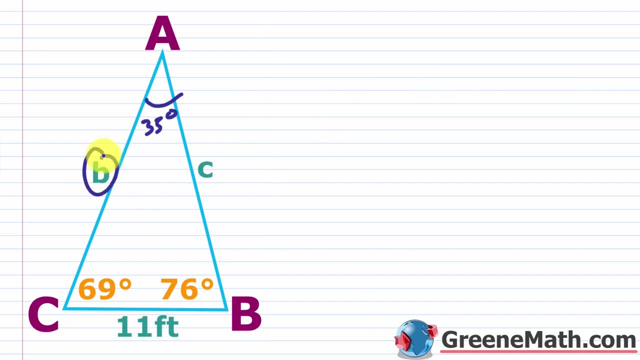 this okay. So now again, if I'm trying to find this guy right here, I say that basically, A, which is 11 feet, 11 feet over the sine okay Of A in this case is 35 degrees. So the sine of 35 degrees is equal to. you'll have this lowercase. 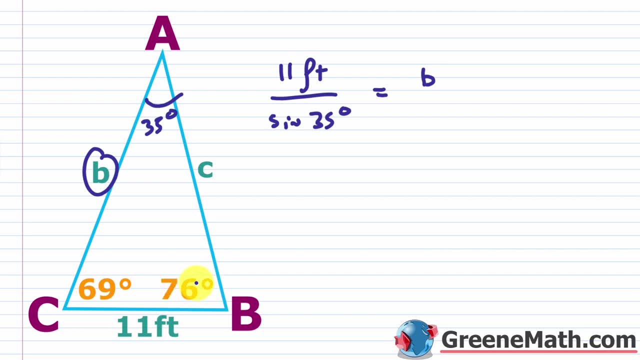 B. Again, it would be over the sine of 76 degrees. but we know we're just going to multiply this by the sine of this angle measure here, which is 76 degrees. okay, So basically I'd have the sine of: 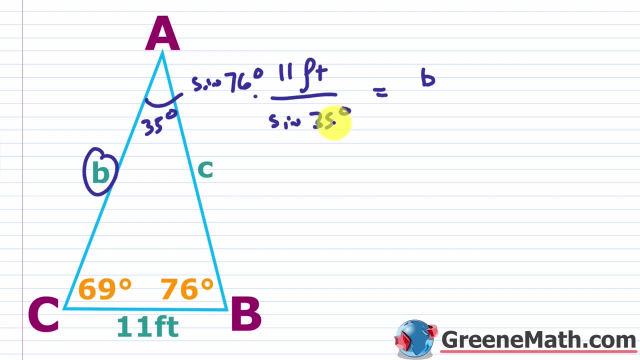 76 degrees times 11 feet over the sine of 35 degrees, So that would be about 18.6,. okay, So let me erase all of this and I'm just going to say- I'll just put this up here- that this guy right here is about 18.6, and this is in terms of feet. 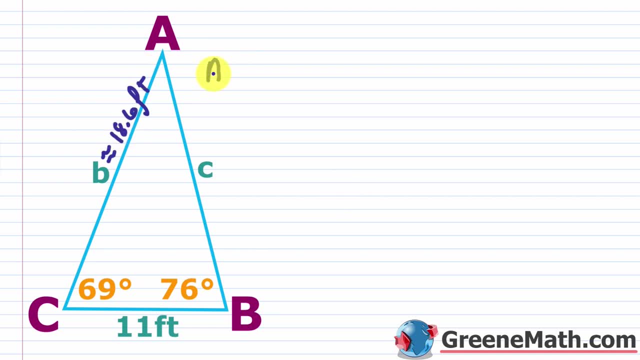 So now it's really easy to go back to our problem. We're going to say that the area okay is going to be equal to one half times again. I'm taking this guy right here, which is the 18.6, okay feet, and then times this guy right here, which is the 11 feet okay, And then times 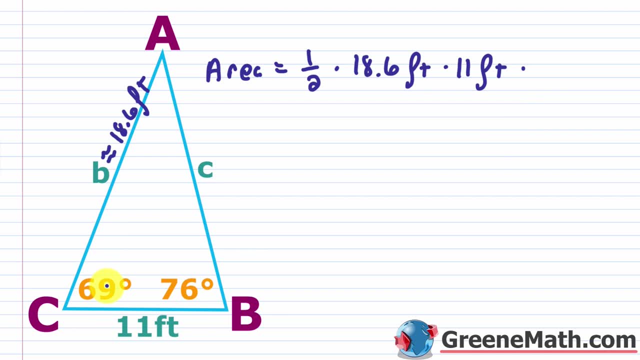 the sine of the angle, okay between them. So in this case it's 69 degrees. So times, let me do the sine of 69 degrees, okay? So let's just punch this into a calculator. So if I round this to the 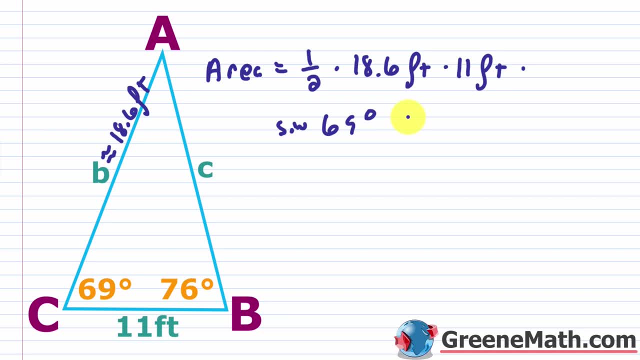 nearest tenth, I'm going to say this is about 95.5 feet squared. okay, or square feet, however you want to say that. So let's go ahead and say this is about about 95.5 feet squared, or again. 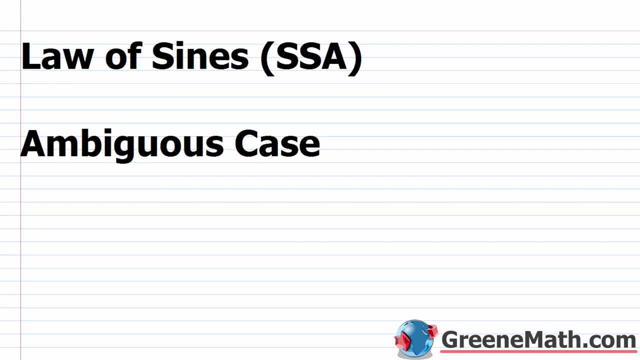 square feet. however you want to put that. In this lesson we want to talk about the law of sines, where we have the ambiguous case. what's given is the SSA or the side-side angle, All right. so in the last lesson we talked about how to basically 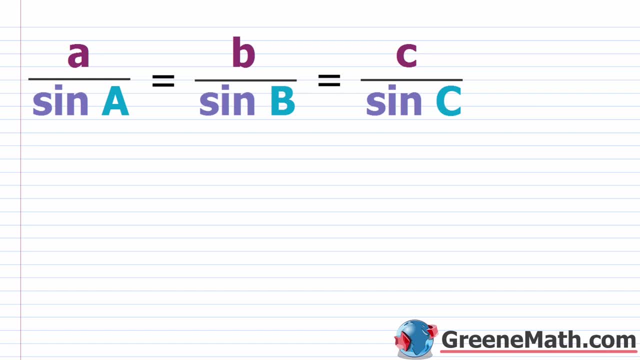 solve these oblique triangles. these are non-right triangles when you're given two angles in one side. So this could be angle-side-angle, which is ASA, or it could be side-angle-angle, right, SAA. Now that's the easy case. you just go immediately into using the law of sines. okay, you can just. 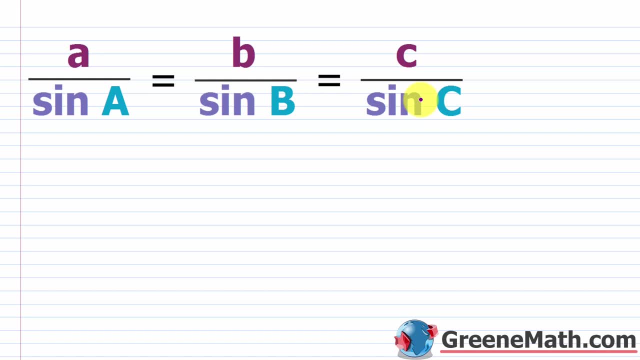 basically set up these proportions and you can solve for what you need to solve for. So you're going to see side-side angle and now you have to dig into the details of the problem. So before I get started into that, I just want to recap some things that we're going to need for. 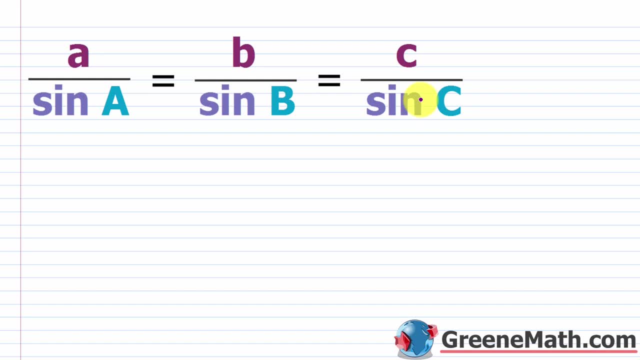 this lesson. Some of you might find this quite boring, so you can just skip ahead to the examples, but I think you might find it quite beneficial. Okay, so, first and foremost, let's revisit the law of sines. We have this: A over sine of A is equal to B over sine of B, which is equal to C. 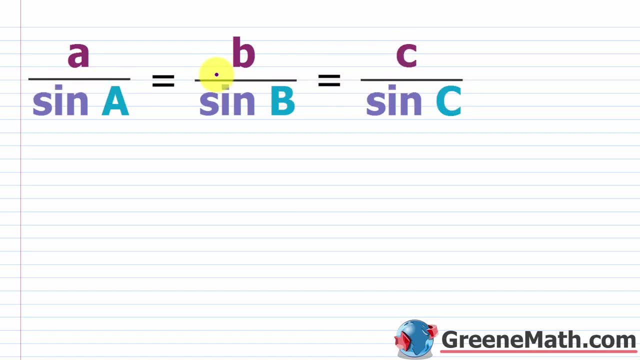 over sine of C, So we just write this in a compact form. You're only going to use two of these at once, right? So you might set these up, and you're going to have a lot of different options, So you're. 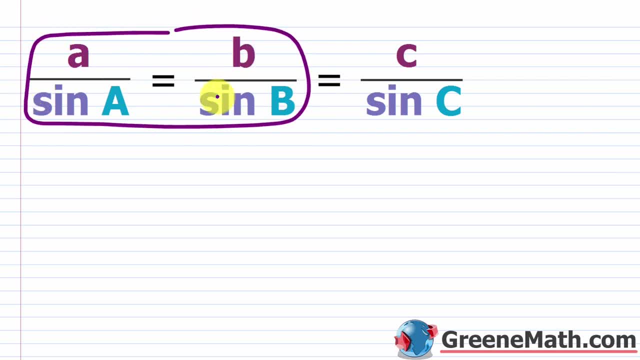 going to have a lot of different options. So you're going to have a lot of different options, So you're going to set these two equal to each other, like this: okay, if you're trying to solve for something in there, or you might set these two equal to each other, or you might set this one and this one equal to each. 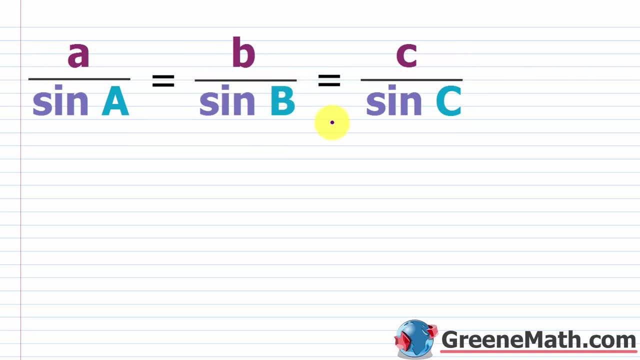 other, whatever you need to do. okay, so you're basically going to use two at one time now. alternatively, you could also write this like this, so you could say: the sine of a over a is equal to the sine of b over b, which is equal to the sine of c over c. now, really quickly, because i know. 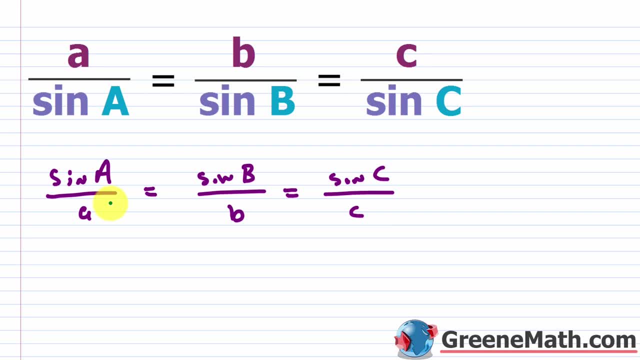 somebody's going to be confused. remember we name the triangles, okay, generally speaking, you'll see triangle a, b, c in your textbook. so capital letter a, capital letter b, capital letter c- remember those are angles. okay, the lowercase counterparts. in other words, if i think about capital letter a, 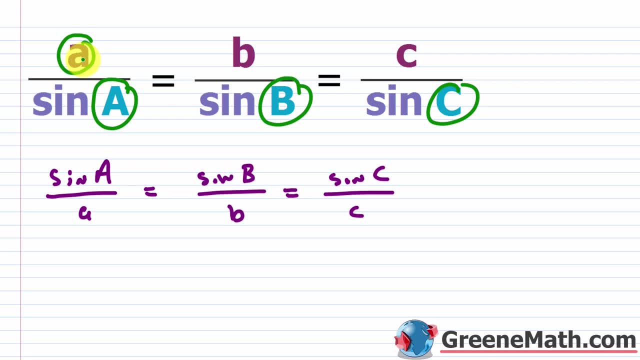 and lowercase a. the relationship is basically: the lowercase letter is going to be opposite of the angle. okay, that's named with that capital letter, so you have capital letter a. if i look at lowercase a, that's going to be the side opposite of the angle. okay, that's named with that capital letter, so you have capital letter a. if i look at 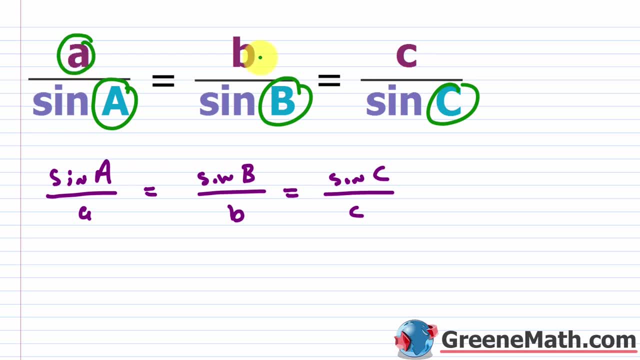 that angle. okay, it's going to be the length of that. if i look at lowercase b, it's going to be the side opposite of this angle. okay, with capital letter b, that's the name of then. if i look at lowercase c, it's going to be the side opposite of this angle, named with an uppercase c or a capital. 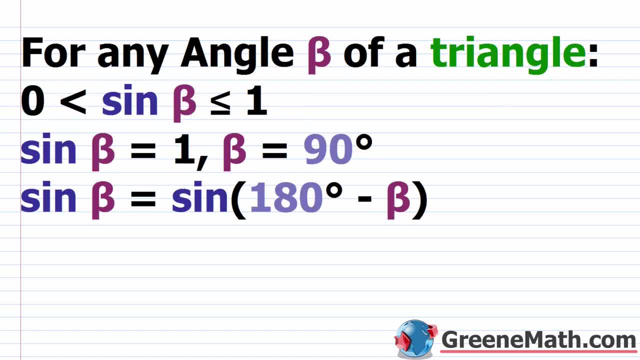 i c. however, you want to say that now let's think about some of the properties for an angle. let's call it beta of a triangle, okay. so this is really important when you think about the sum of the angles in a triangle. we know it's 180 degrees, okay. we know we can't have an angle in there. 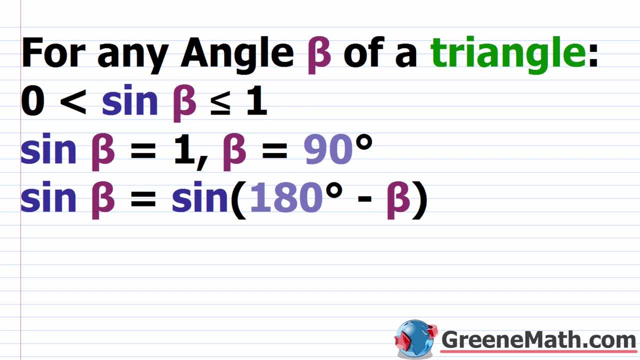 that's going to be zero degrees. it's going to be not possible. and also, we can't have an angle that's 180 degrees. that's not possible as well. so we know that the sine of beta has to be greater than zero. okay, it can't be zero because, again, you can't have a zero degree angle. okay, and you also. 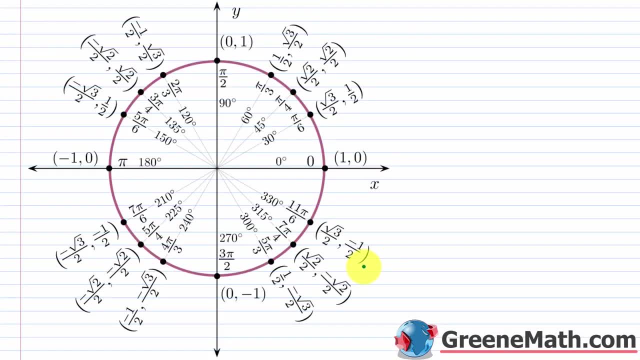 can't have an angle that's 180 degrees. if we go back to the unit circle, remember, if you think about a sine value of zero, it's going to happen, basically, if your angle is zero degrees or if it's 180 degrees, and i just said that's not possible. okay, so we go back, we think about the 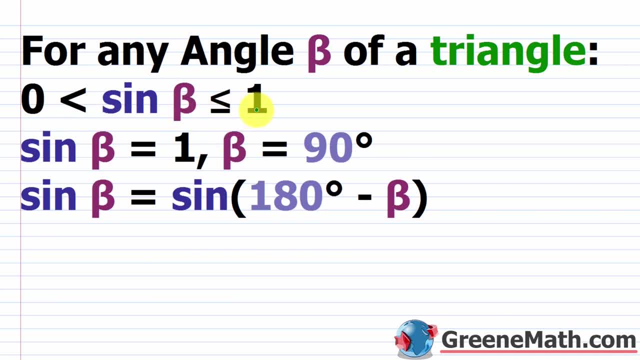 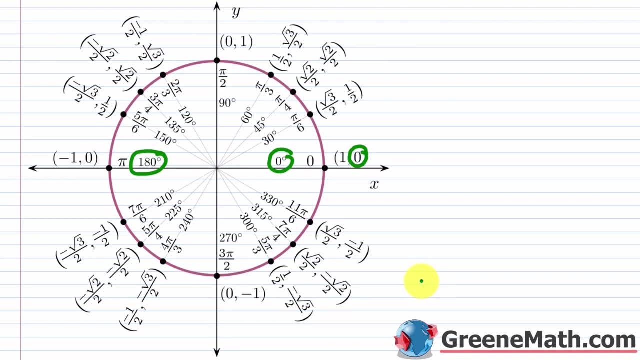 next part of this. the sine of beta is again greater than zero and less than or equal to one. remember, when you think about the sine. okay, we know the range of sine in general is from negative one to one, but again, if you're working between zero and 180 degrees, not including zero or 180, 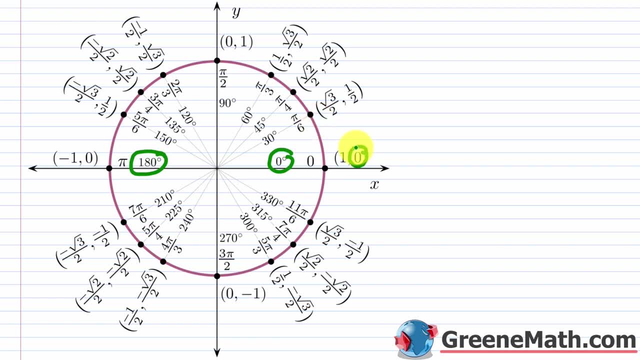 well then, basically, you're going to be between zero and one, where zero is not included, and one is right. if you have a 90 degree angle where you can have a sine value of one, okay, that means you have a right triangle. so let's go back here. i said sine of beta equals one. if this is the case, 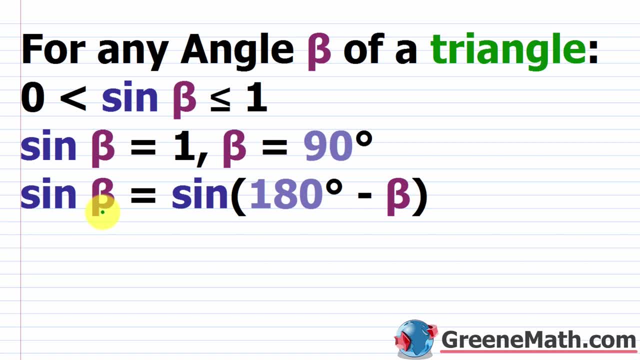 again, you have a right triangle. lastly, we need to understand this because when we have two solutions here, this is going to come in. so remember the concept of a reference angle. if you have sine of some angle, beta, let's call it 30 degrees. so sine of 30 degrees, this is equal to sine of 180. 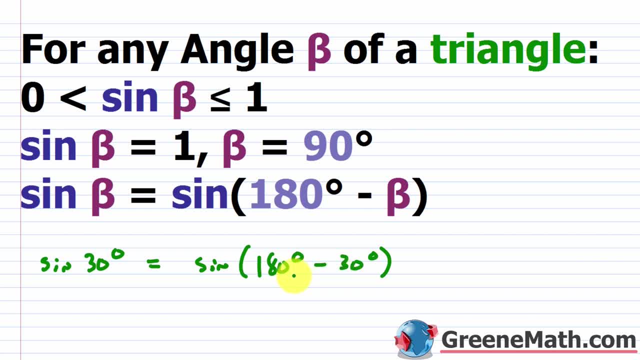 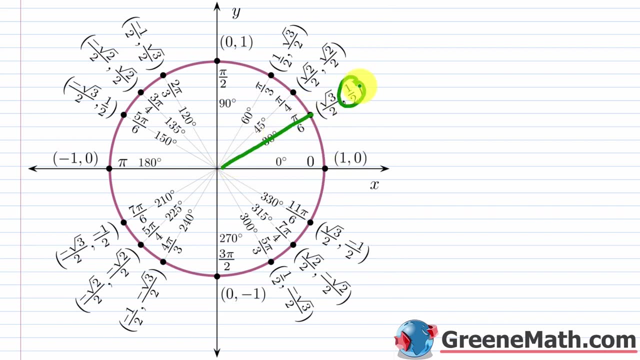 degrees minus 30 degrees. okay, 30 degrees here. if i take that away from 180 degrees, this would be 150 degrees. so this is sine of 150 degrees. we know this is true because of the concept of a reference angle, and so let's say this is the case here. if i had a 30 degree angle, the sine value is a half. 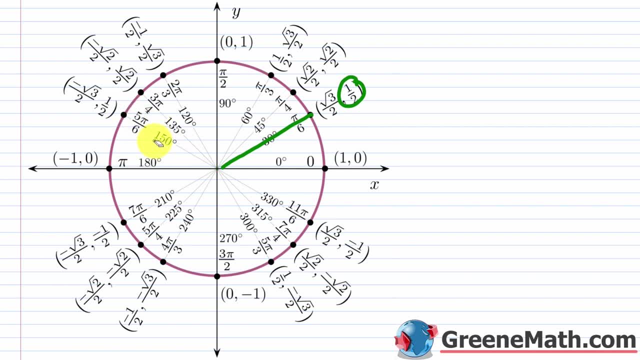 if i had 150 degree angle. okay, and i didn't draw that really well, so let me try that one more time. the reference angle there is 30 degrees, so the sine value is also a half. okay. again, this is going to come up in a moment because we're basically going to be using the inverse to find 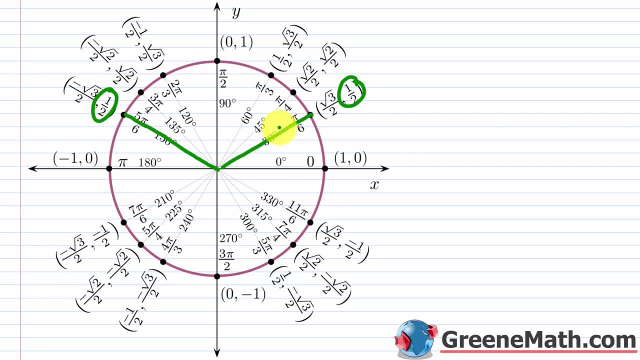 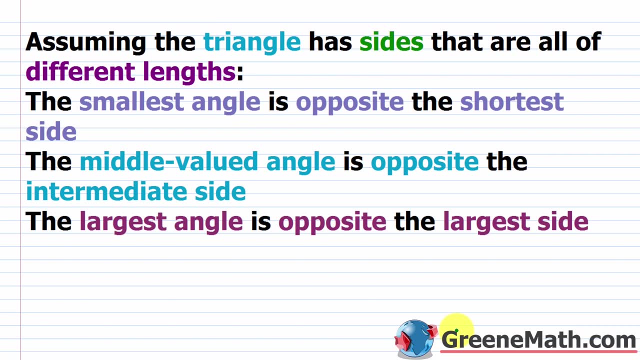 our missing angle measure, and it might be possible that we have one that's, let's say, 30 degrees and another that's 150 degrees. okay, so we need to keep that in mind. now just a few other quick things. assuming the triangle has sides that are all of different lengths, the smallest angle is going to 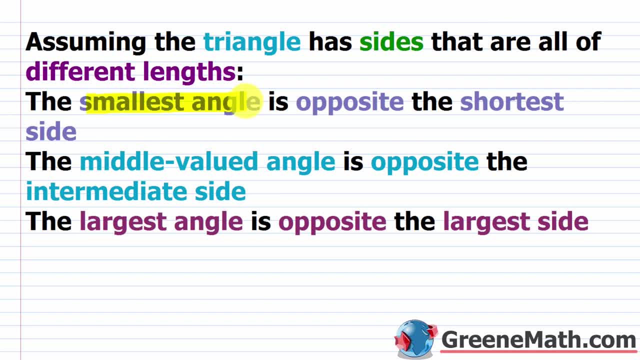 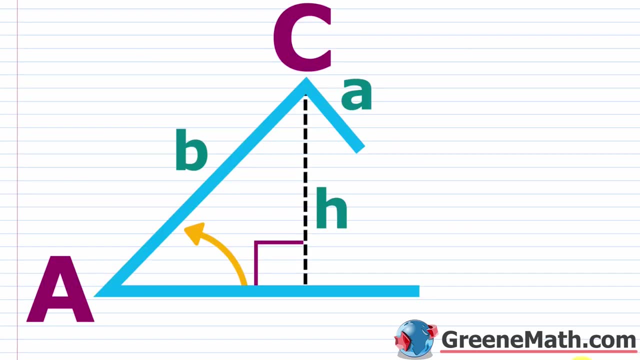 be opposite the shortest side. let me highlight that the smallest angle is opposite the shortest side. the middle valued angle is opposite the intermediate side. the largest angle is opposite the largest side. okay, so you need to make sure you understand that, because again it's going to come up today. all right, let's jump in now and look at some examples. i'm going to go through all the 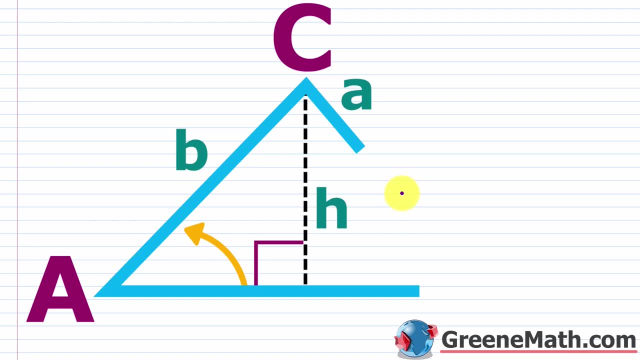 different scenarios and give you an example of each. so the first thing we're going to look at would be where there's no such triangle and you're given an acute angle. so we're given some acute angle, a, and remember, opposite of a. we're going to have this side here, which is named with. 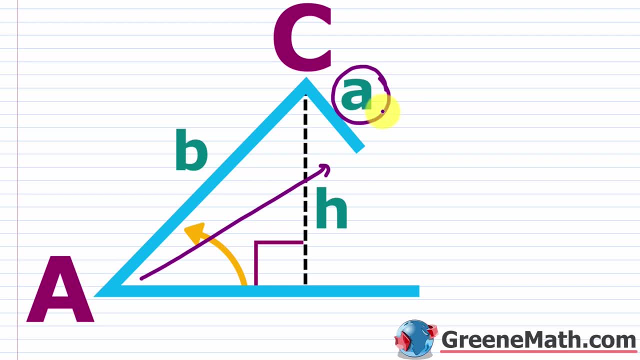 lowercase a. so we're given some angle a and then, opposite of that, we have some side a. these are both going to be given to us. we're also beginning, given this side b here. okay, so the first thing you could think about: if you wanted to show that there was no such triangle, you could say that h is going. 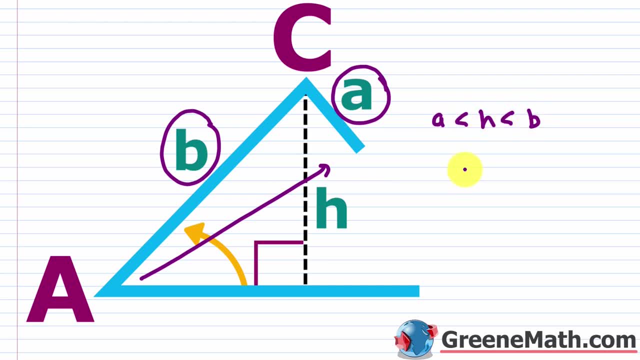 to be greater than a and it's going to be less than b. okay, so you could prove it that way. so this way you could also show that the sign, okay, of this guy b. if you try to set this up with the law of sines, you're going to end up with something that's greater than one. okay, so i'll show you both. 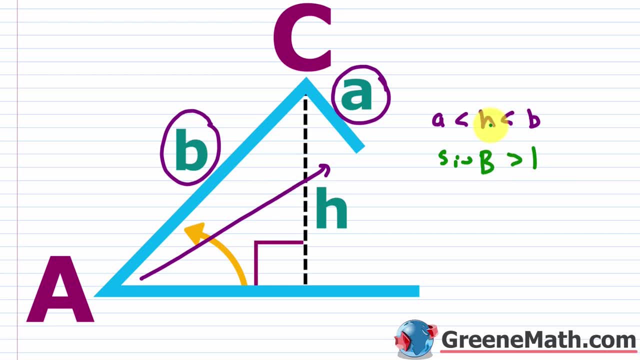 for this example that's coming up in a minute. now you might be thinking: how in the world am i going to get h? so let's talk about that real quick. let's get rid of this. okay. let's think about if we formed a right triangle here. okay, we thought about this angle a. well, the sine of a is equal to what it's. 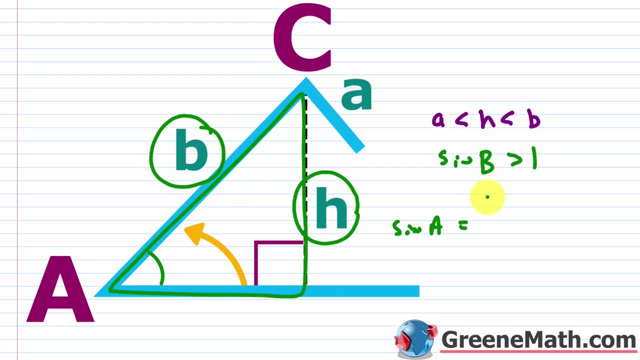 hypotenuse. so in this case, because i formed a right triangle here, the opposite of it is h and then the hypotenuse is b. okay, if you wanted to solve this for h, you would say that h is equal to b. okay, whatever, this side is here times the sine of a. the angle that you're given, okay, this. 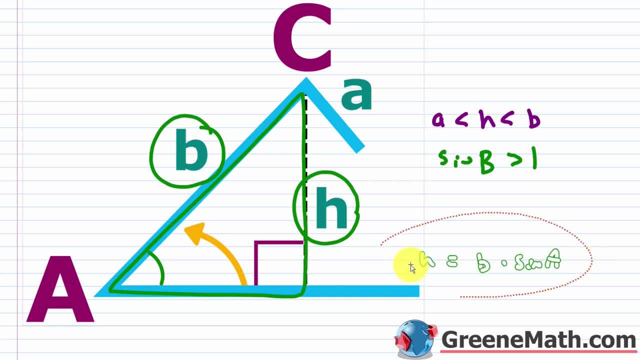 is pretty easy to remember. it's going to erase this real quick and just drag this up here. let me go down and we'll read off our problem and we'll come back and we'll just kind of use this as a visualization of it. so we're given here that. 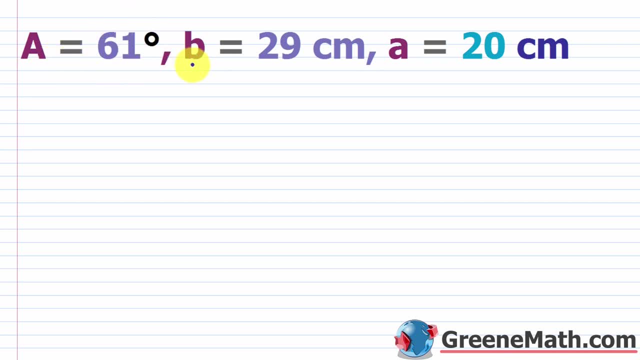 a is 61 degrees. so notice, this is an acute angle, right. then b is equal to 29 centimeters and a is equal to 20 centimeters. so again, this is your angle here. and then this right here, because it's the lowercase letter counterpart: this is the psi. that's opposite of that. okay. so when we set this, 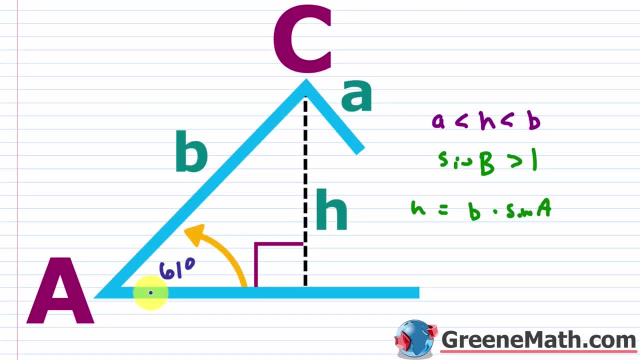 up, we'll say: this is 61 degrees. okay, that's the angle you're given. opposite of that, you have this side. let's just go ahead and say again: it's a, so this is 20 centimeters. and then b, we're told this is we'll get a 25 around this point. okay, so h- the sin, the sine, and a right here, and we're going to. 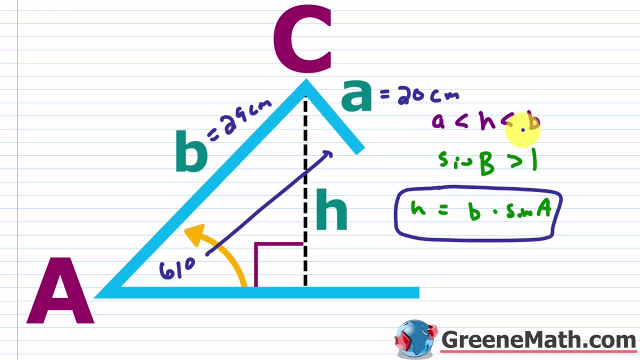 get b of b and h of b and h of b and b. write them down here, okay, so let's take h of b, ii and a g of c and this little part here. this little part here is a sine of b and this is the amplitude that you. 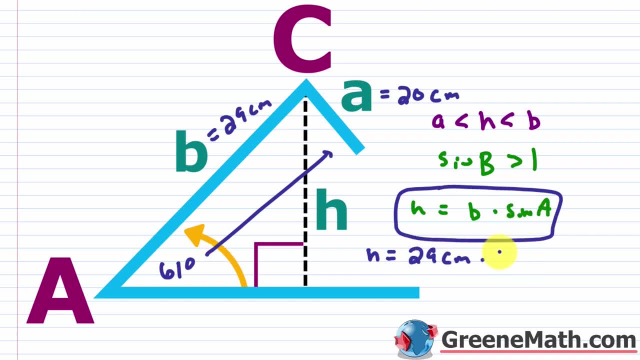 wanted to get here and then you cut out this out of your chi. this is the intra along and ii. here is the integral sin of rk at the top here. so we're actually going to have a single cosine of i tale concept right here with our. we're gonna have b at the cap. at the end there's a sine degreeٍ, because 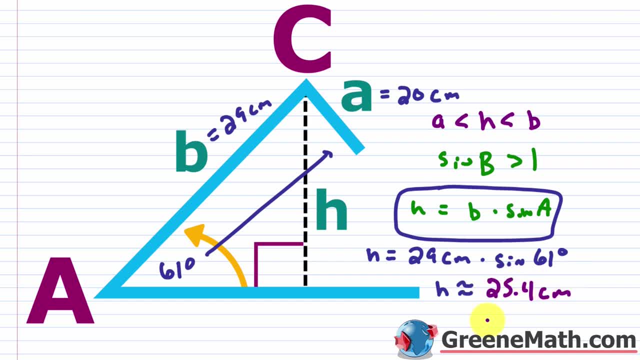 that's what, what exactly I have here, and a is bitcoin over块. you can get those things right here, okay. I mean the inscrement queues up here in the bottom part of this fueling, we're going to get in the bottom 25.4 centimeters, Okay. So you can see here that it basically, if I set up this inequality- 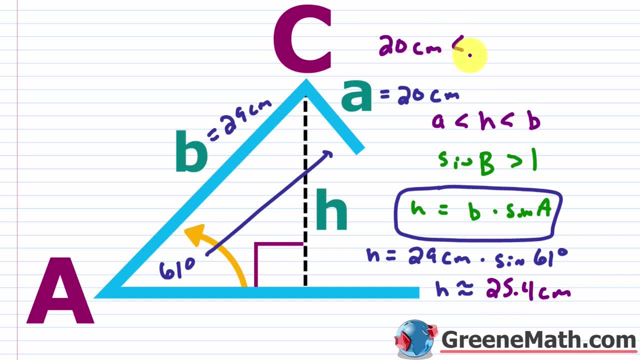 I could say that 20 centimeters, which is a, is less than 25.4 centimeters, Okay. Which is H, is less than you could say 29 centimeters, which is your value for B, Okay, So we fall into this. 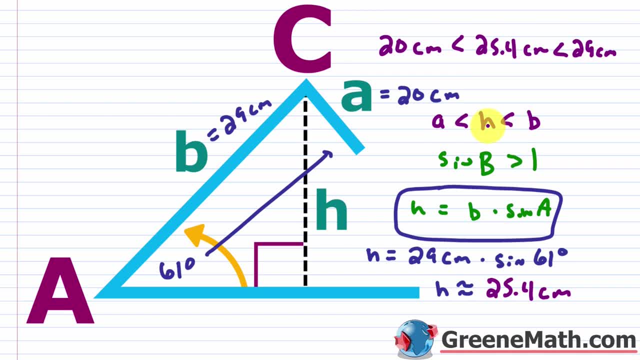 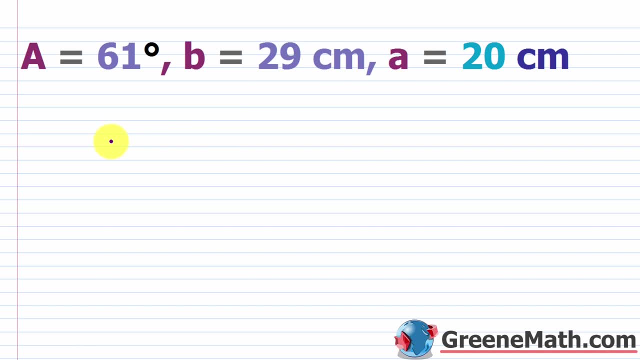 case here, or we could say: there's no such triangle, It's not possible. The other thing you can do- and let me just erase this: If you wanted to do it this way, you could say basically that the sign, okay, the sign of this angle here, 61 degrees, Okay, So the sign of A. 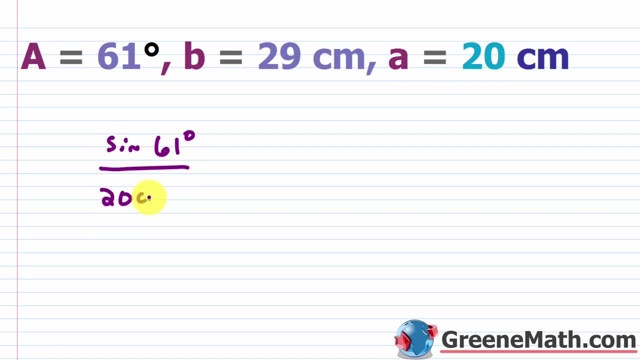 over A itself, in this case is going to be 20 centimeters- is equal to, again, the sign of this angle B over this B measure here, which is going to be 29 centimeters. Now you can multiply both sides by 29 centimeters. Let me just kind of slide this down a little bit, So we'll say times. 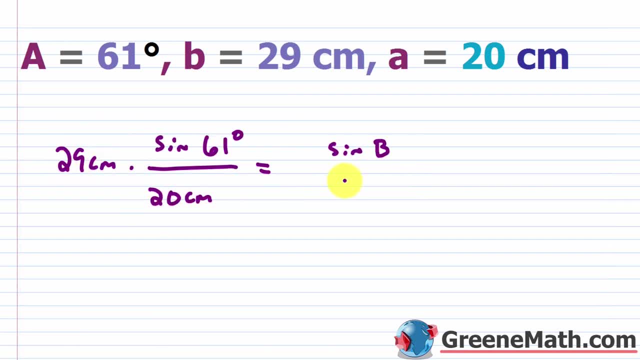 29 centimeters over here. So we'll say this is equal to the sign of B. So the sign of of B is approximately. let's just go ahead and say it's about 1.3 in terms of this guy And again. 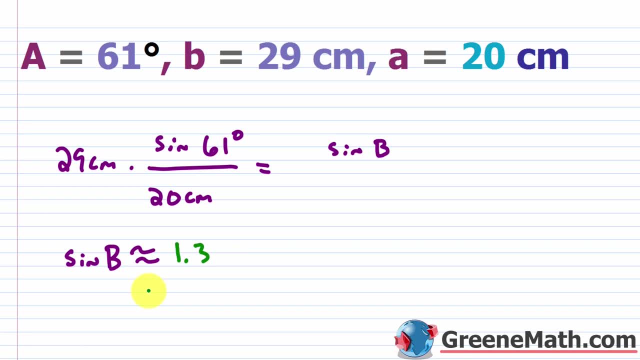 the sign value is not going to be greater than one. So that's another way you can prove that there's no such triangle. So, however you want to do it, basically, if you're going through the process of trying to solve the triangle and you get something that doesn't make any sense, 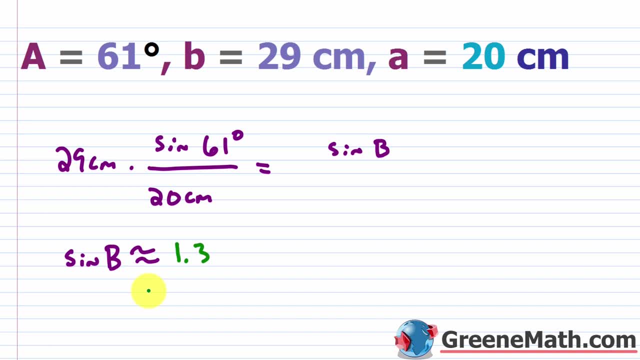 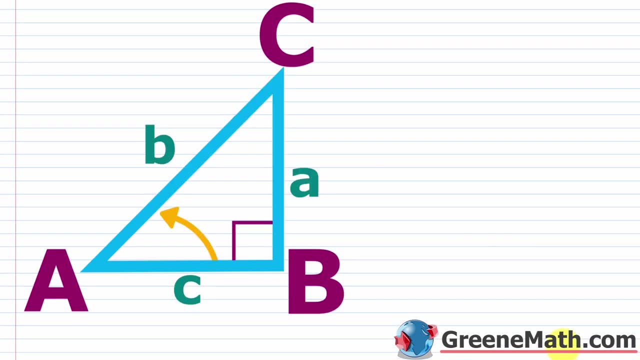 it's just nonsense. You want to stop and say no such triangle? Okay, So let me just put this over here and just say no such triangle. All right, Let's look at another scenario. This is one where you end up having a right triangle. So basically, here you're going to see that this A value here. 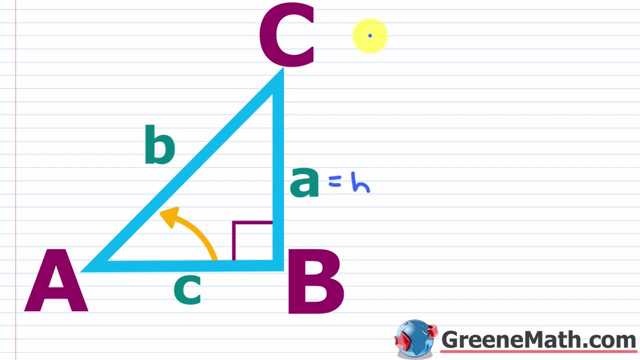 is exactly equal to H. Okay, So if A is equal to H, and then you could also say either A or H, because they're equal, let's just go ahead and say A is going to be less than B. Then we know that we. 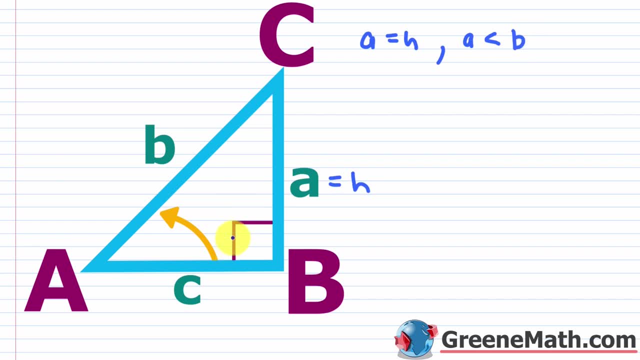 have a right triangle. Now another thing here: since you notice you have B as a right angle, you could say that the sign of B- remember this- is going to be equal to one. So two ways to kind of check this. Let's go ahead and look at our example real quick. So we have: A is 30 degrees. 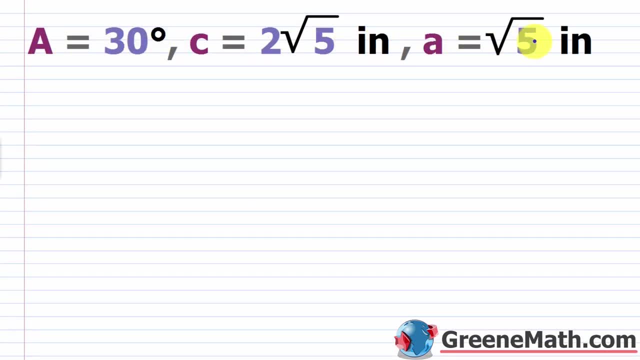 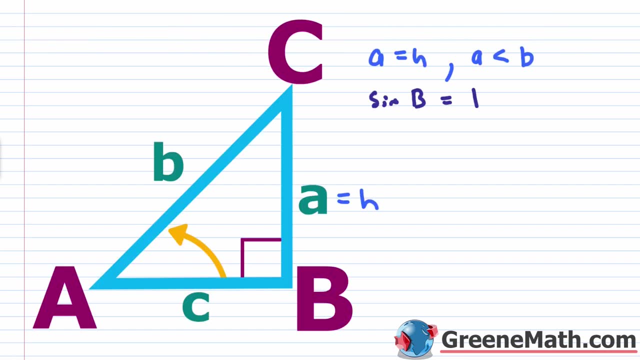 C is equal to two times square root of five inches And A is equal to the square root of five inches. Now, instead of giving you a letter B, I gave you a letter C, just to throw a wrench at you. This is not any harder. If you want to work with this, on this particular image, you just need to. 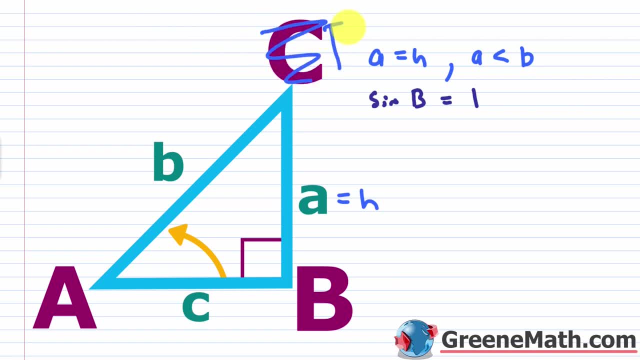 cross this out. Let me use a lighter color. You need to cross this out and put capital letter B. cross this out and put capital letter C. cross this out and put lowercase C. cross this out and put lowercase B. Just adjust for what you're given. They're not always going to give you things in the exact 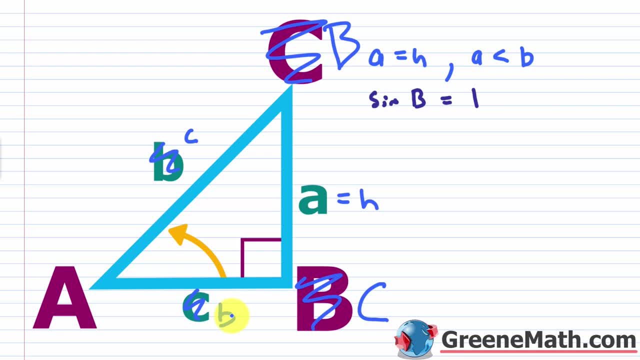 format. it is in your book. So the first thing is: I want to prove that A is equal to H. How do I do that? Well, I'm given that A is equal to the square root of five inches. I'm given that, and I messed. 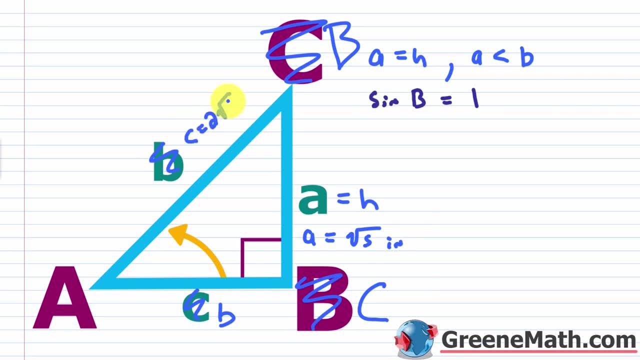 that up. I'm given that C is equal to two times the square root of five inches And I'm given that this angle A is 30 degrees. Now remember, for the height, we can say the sign of the angle A. the sign of the angle A is equal to- again, it's the opposite, which you could use as H here. 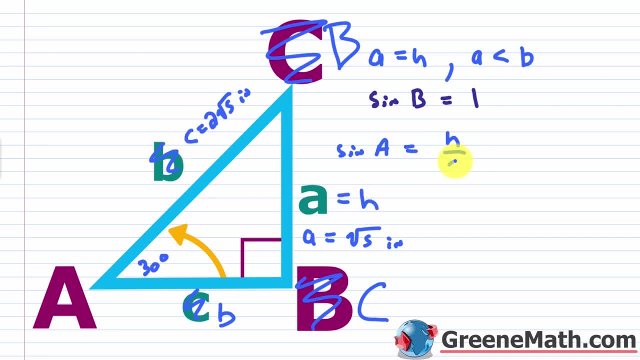 okay, over the hypotenuse, which in this case, we're going to use C. okay, So basically, H is going to be C, times the sign of A, So H. you can write this over here: H is going to be C. 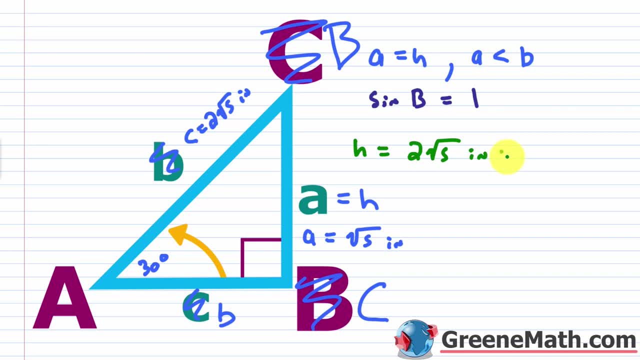 which we know is two times square root of five, two times square root of five inches times the sign of. in this case it's 30 degrees, right, The sign of A. So what is the sign of 30 degrees We? all know from the unit circle: it's a half. So what is the sign of 30 degrees? We all know from the unit circle: it's a half. So what is the sign of 30 degrees? We all know from the unit circle: it's a half. So let me put a. 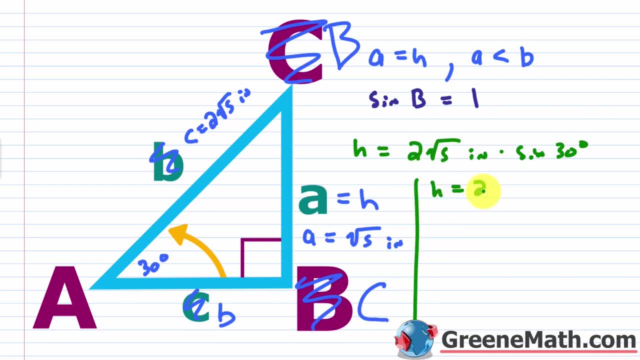 little border here. H is going to be equal to two times the square root of five inches, times one half. okay, My writing is getting a little sloppy here, So let me change that and put inches there, so we know, or actually I can move this out to the end so that we don't have to mess with it. for. 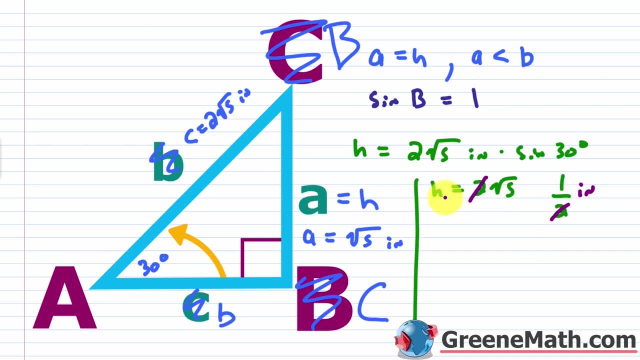 right now We see this two, we cancel with this two And basically H is equal to the square root of five inches. Well, what is A Square root of five inches? So you've already shown that A is equal to H And also you can see that A is less than B In this case. 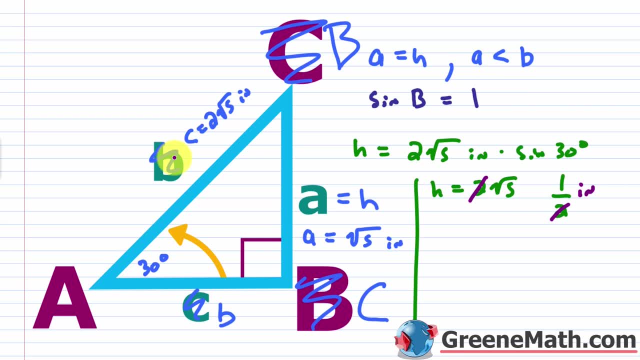 we swapped B and C around, So again, you got to keep that straight in your mind. So this value here- okay- is less than this value over here. That's all you need to worry about Now. in this particular case, you could also show that the sine of this angle- in this case, it would be the angle. 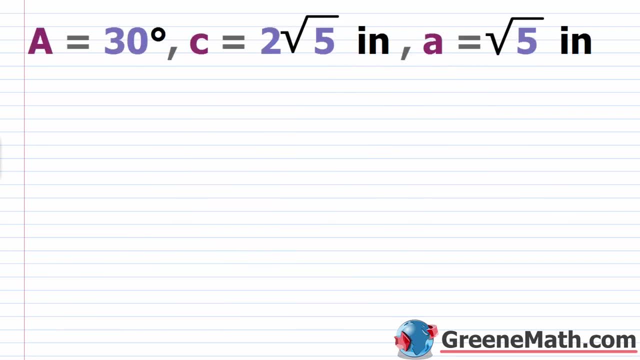 C now is equal to one. So let's go down and think about this. So again you use your law of sines. You could say that the sine of 30 degrees over this square root of five is equal to you would. 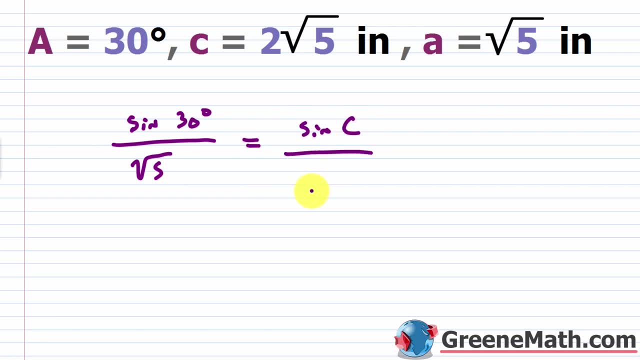 have your sine of C over B. So let's go down and think about this. So again you use your law of two times square root of five. okay, So let's just go ahead and say: this is a half, So I have. 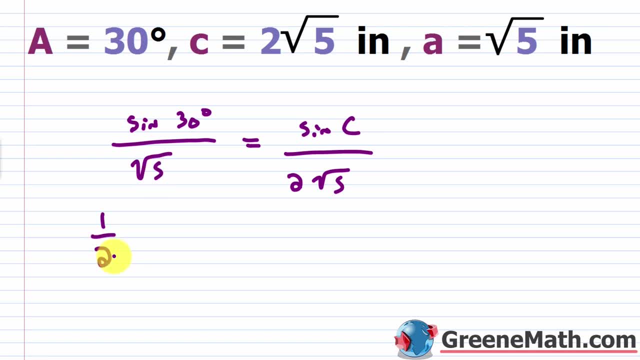 one half, And then I'm dividing by square root of five. So I'll just say down here: it's two times square root of five. okay, So one over two times square root of five, like this, is equal to: I'm going to multiply both sides by this. So I'm going to multiply both sides by two times square. 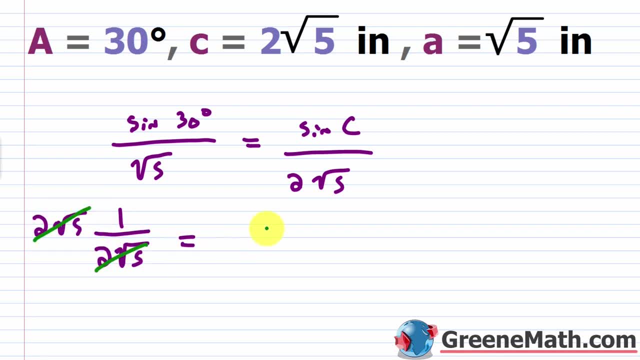 root of five. And so, look, this is going to cancel here with here, And this is going to be equal to the sine of C. So the sine of C is equal to one. okay, So a little rough sketch of this, if you. 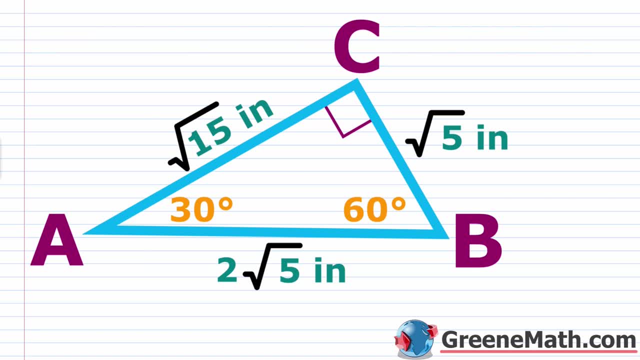 want to look at it Basically. if you want to find the rest of this, you're going to have to do this. So you already know that C is a right angle, right, The sine of that guy is one. We already know that, opposite of that, where we're given that this is two times square root of five, 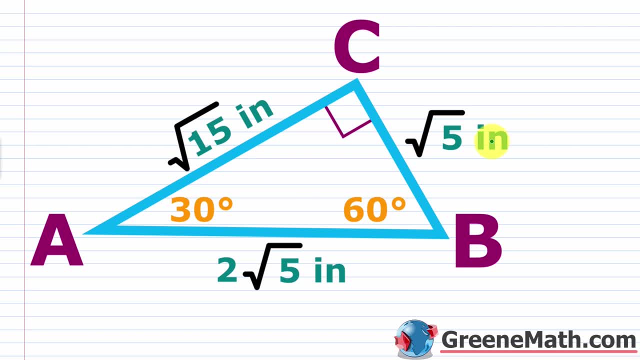 inches. We know A is 30 degrees opposite of that square root of five inches. So we need to find this and this. So where does that come from? If I want to find this 60 degrees here, the measure of angle B, again what I want to do if I come back up here- let me erase this- I would say that 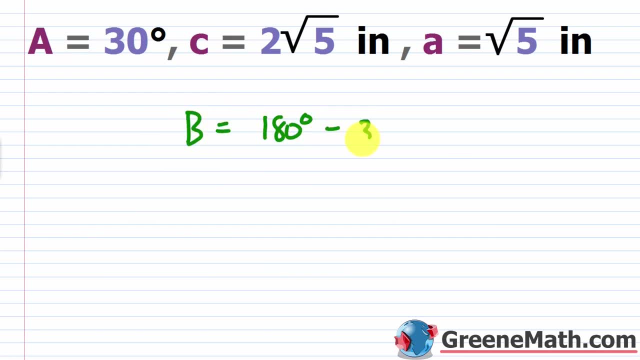 B is equal to 180 degrees minus 30 degrees minus 90 degrees, which is equal to one over two times square root of five. So I'm going to multiply both sides by 60 degrees. right, Remember, the three angles in a triangle have to sum to 180 degrees, So I can. 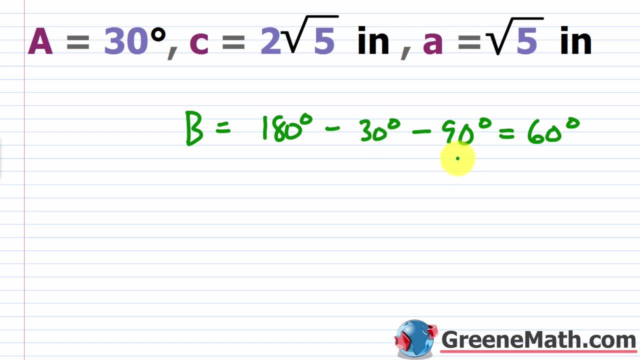 just take 180 degrees minus the measure of one angle, minus the measure of the other angle. That gives me the measure of the remaining angle right, Which in this case is B. So B here is equal to 60 degrees. Now how do I find this lowercase B? How do I find this guy right here? 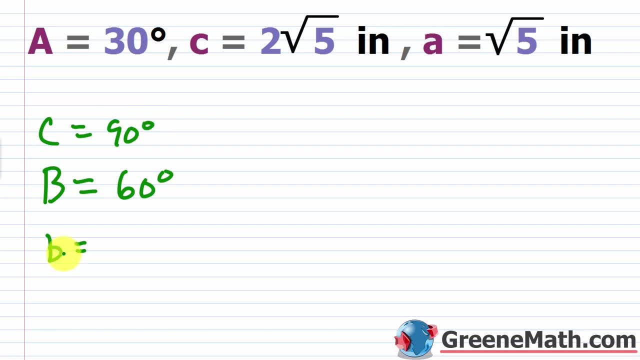 Let me write in here that C is 90 degrees, so we can solve this completely. Well. lowercase B is going to be found using again the law of sine, So I'm just going to go. in this case I'll go square root of five inches over. I'll go the sine. 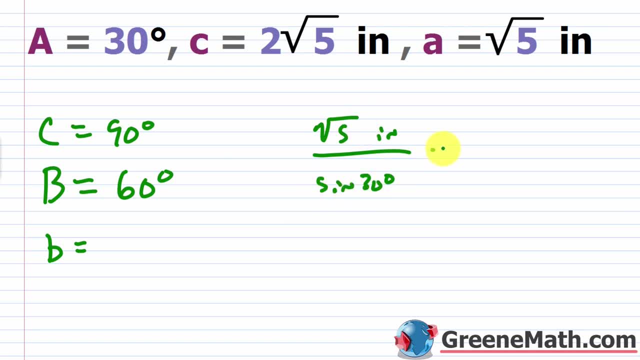 of 30 degrees. So I just did: A over the sine of A is equal to, I'm going to say B, okay, B, which is unknown, over the sine of B. So the sine of 60 degrees, So the sine of 60 degrees, We know the. 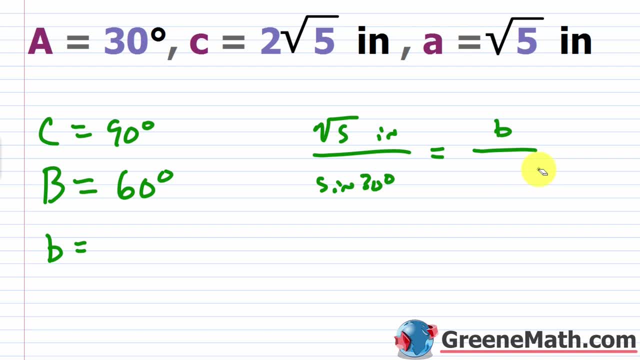 sine of 60 degrees is square root of three over two, right? So let me put this in here as square root of three over two. And we know the sine of 30 degrees is a half okay. So this is a half Okay. 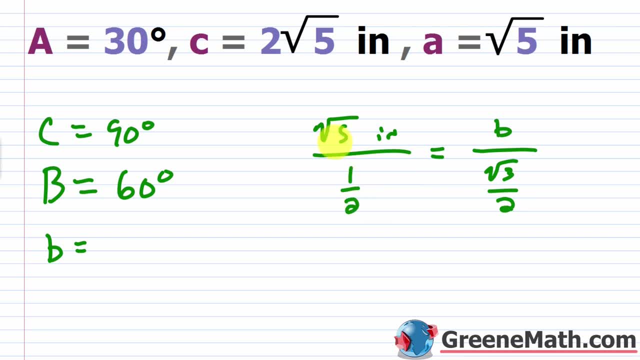 so let's think about simplifying this a little bit. We know this would basically be two times the square root of five inches. okay, if I simplify that. So this would be two times the square root of five inches. Over here, this would be two B over the square root of three. So what I'm going to do to get B? 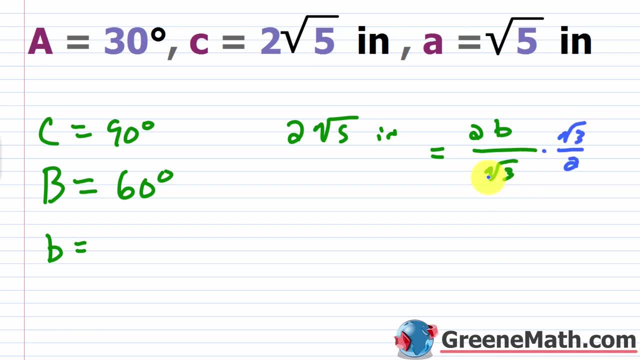 by itself. I'm going to multiply both sides by the square root of three over two, So this will cancel and this will cancel, okay, And over here, square root of three over two, So this is going to cancel, And basically you get that B is equal to square root of three times square root of five. 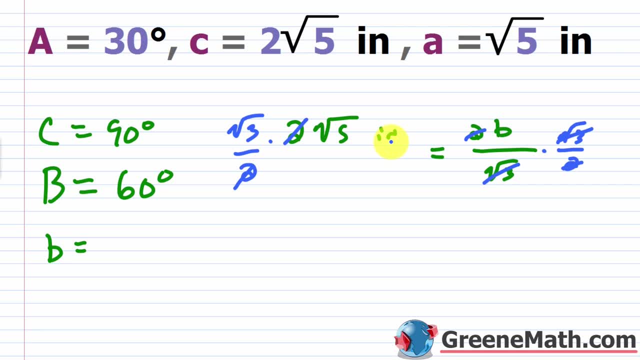 inches, which I could write as a square root of 15 inches, Right? So basically, B is the square root of 15, okay, inches. So let me erase this. And so now we've solved the triangle, right? We know all the sides and all the angles Again, if you go back. 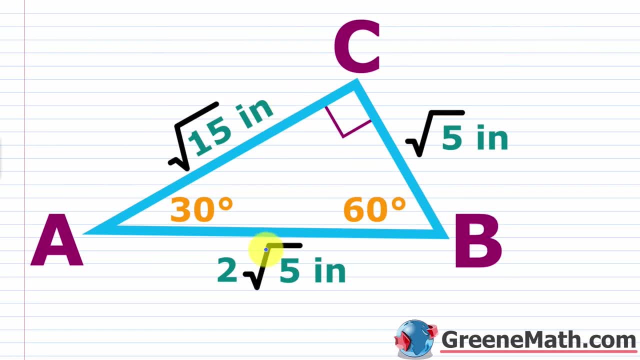 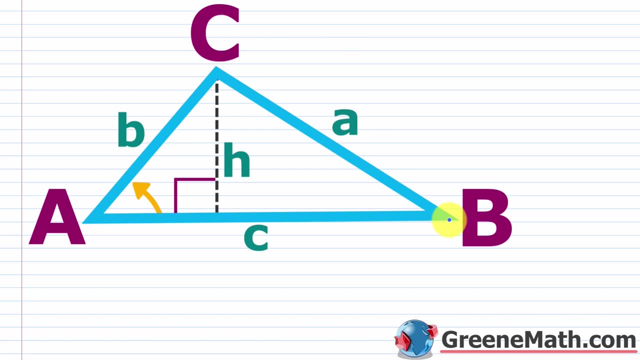 to this little picture here, or this little image, whatever you call it. again, this is 60 degrees, that's for B, And then the side opposite is square root of 15 inches. All right, let's look at another scenario. So this will be our third scenario. So here you're going to see that. 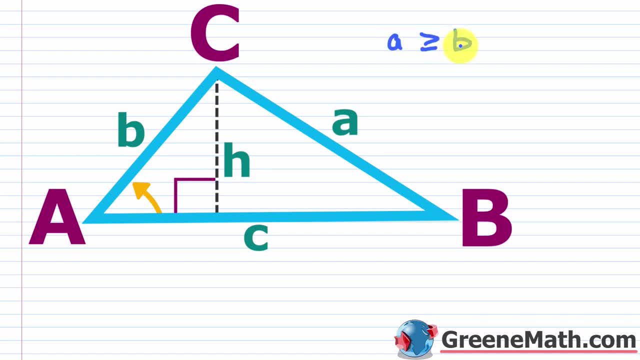 basically, your A is going to be greater than or equal to the square root of 15 inches, And so you're going to have exactly one triangle. okay, So you can also say that zero is going to be less than your sine of this angle here. B, okay, which is going to be less than one. okay, It can't be. 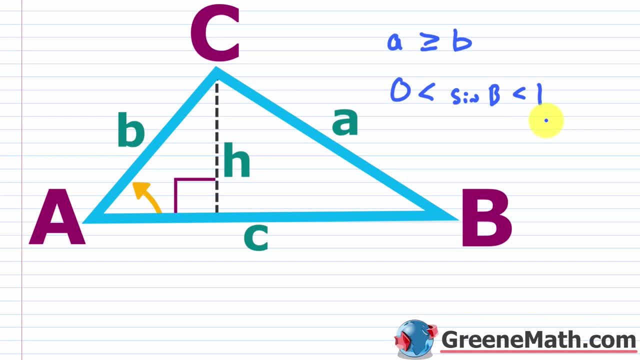 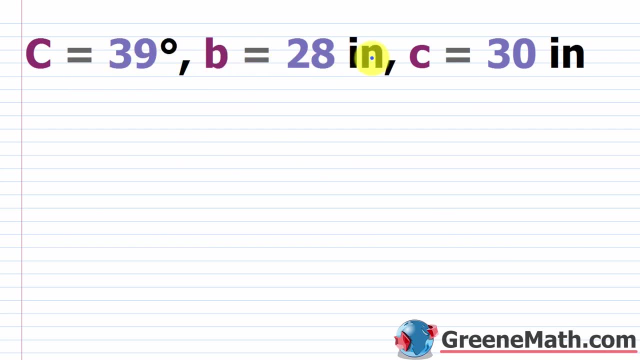 equal to one, because you don't have a right triangle in this particular case. Okay, so let's go ahead and look at an example. And so we have: C is equal to 39 degrees, B is equal to 28 inches and C is equal to 30 inches. Now again, I switched the letters around on you. 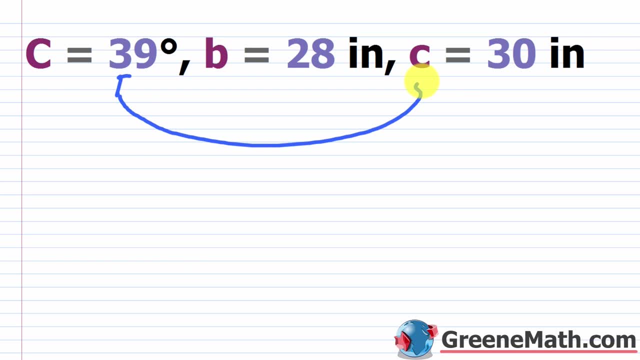 don't freak out. So this is your angle that you're given This side here, lowercase c is the one opposite of that. okay, So you just plug back into the diagram that you're looking at, But for this one you really don't need it If you notice that this guy right here, okay, this. 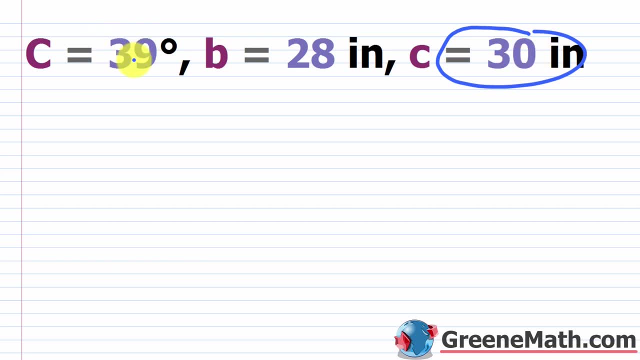 right here is 30 inches. it's opposite of the angle you're given. If this measurement here, which is 30 inches, is greater than or equal to this measurement here, you know you're in the scenario where you're going to have exactly one solution and you just start pounding away at it. 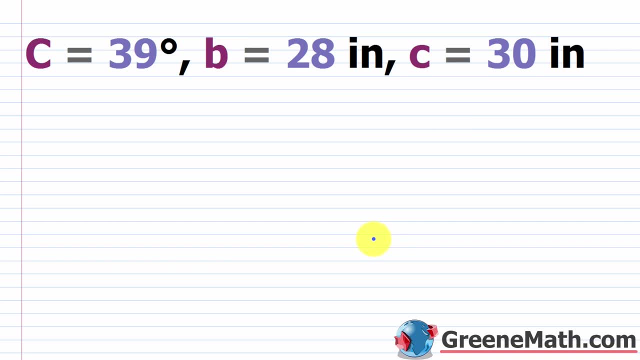 okay, You don't need to do anything else. So the first thing I'm going to do is I'm going to solve for my angle B, So let's start with that. So I'm going to say that the sine of B over B- okay, is equal to the sine of C over C. okay, We know, we can multiply both sides. 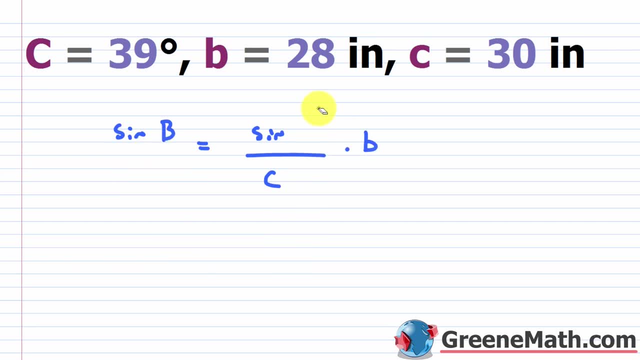 by B here. okay, So you just get rid of this and then I can just plug in: What is C? It's 39 degrees. Let me change my color here. so this is 39 degrees. What is lowercase c here? It's 30. 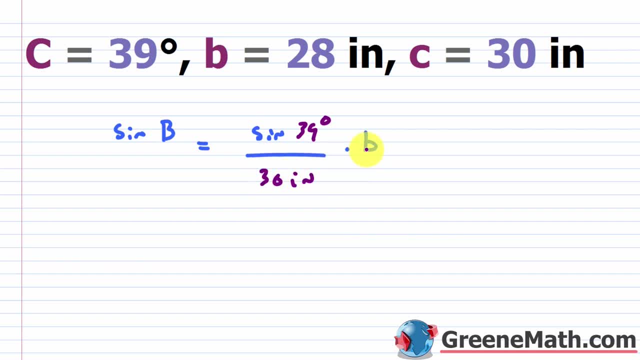 inches, so this is 30 inches, okay. And then what is B? It's 30 inches, so this is 30 inches, okay. And then what is B? It's 30 inches, so this is 30 inches, okay. And then what is B? It's 30 inches. 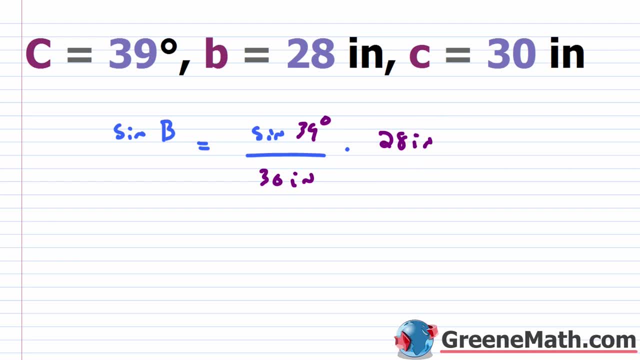 it's going to be 28 inches. okay, If you want to cancel the units visibly, you can, so this is going to cancel. So basically, let me make this a little bit better. okay, So this is 30 right there. Basically, you punch this into a calculator and you need an approximation. So 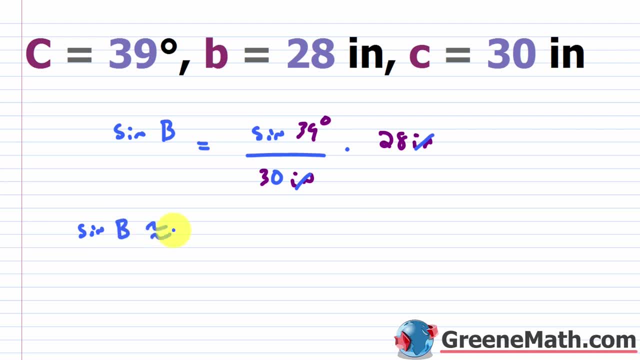 you say sine of B is approximately, I'll say 0.5874.. So 0.5874.. And I'm using more decimal places here because I'm going to take the inverse. okay, So to find B here, you want to. 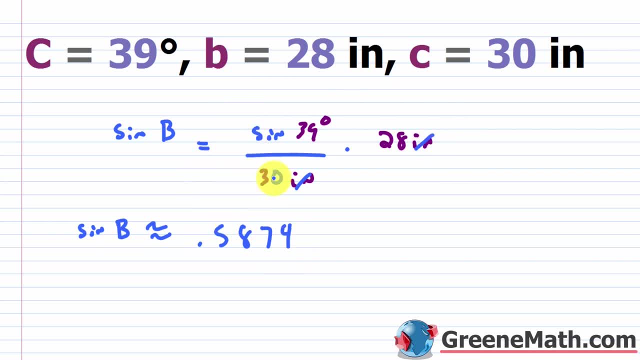 you could wrap this entire thing in parentheses here. so this entire thing here, plug it into the calculator, go sine inverse of that, or you can do this this way You're going to be close enough. So I'll go ahead and say sine inverse of this guy right here: 0.5874, is going to be approximately. 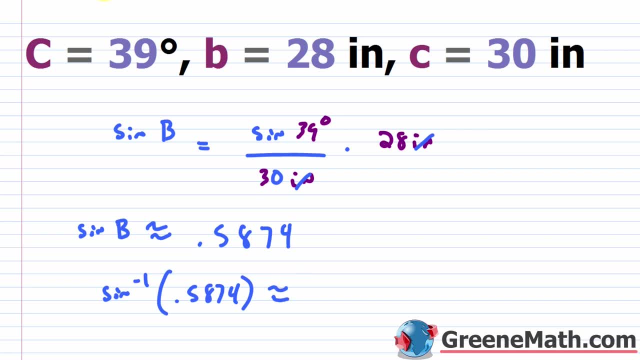 we round it to the nearest tenth. let's just say it's 36 degrees. So let's go ahead and say this is 36 degrees, and again, this is going to be my B here, okay, So let me erase all of this. 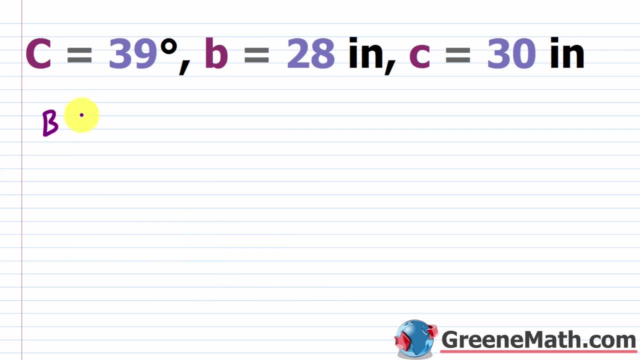 and I will go ahead and say this is 36 degrees. So let's go ahead and say this is 36 degrees and say that B is going to be 36 degrees. okay, And this is approximately. so let me make the approximately symbol here. So then, what is A? I'm solving for A here. Again, this is pretty easy. 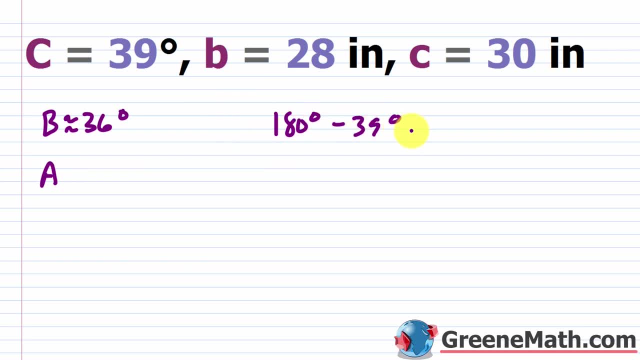 I'm going to do 180 degrees minus 39 degrees minus 36 degrees. This is going to give me what? So 180 minus 39 is 141.. Take away 36, you get 105.. Again, this is an approximation. okay, It's not. 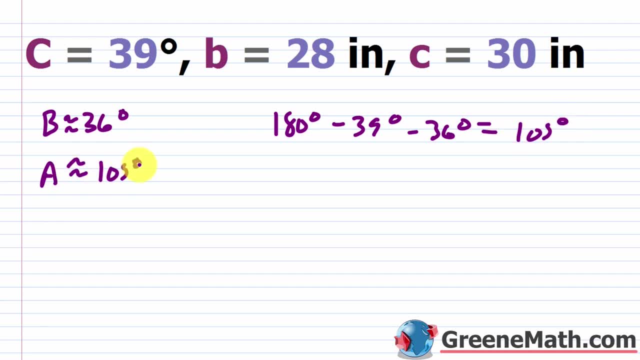 going to be exact. So let's say this is approximately 105 degrees, and if I want the lowercase a here I can just use the law of sines again. So again, go with what you know. So I'm going to go. 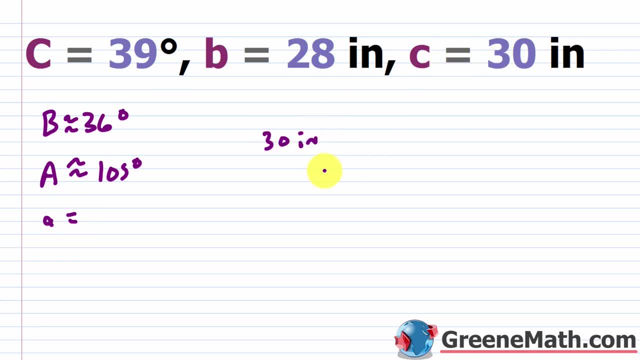 that 30 inches, which is this lowercase c over the sine of 39 degrees. So the sine of 39 degrees again, the sine of c- Let me make that better- I'll say is equal to: you're going to have your. 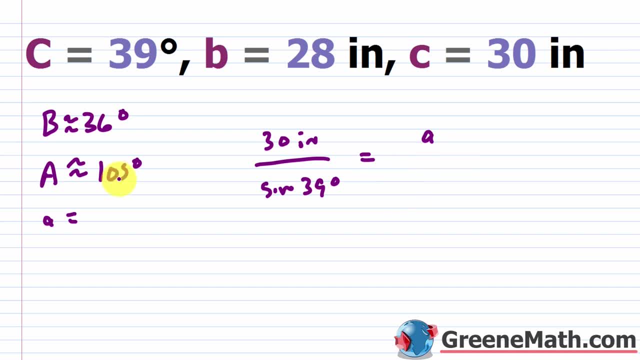 lowercase a over your sine of 105 degrees. Again, I'm going to multiply both sides by the sine of 105 degrees, so I might as well just do it over here. So the sine of 105 degrees. So again, remember, this is an approximation, So let's go ahead and say this is approximately. 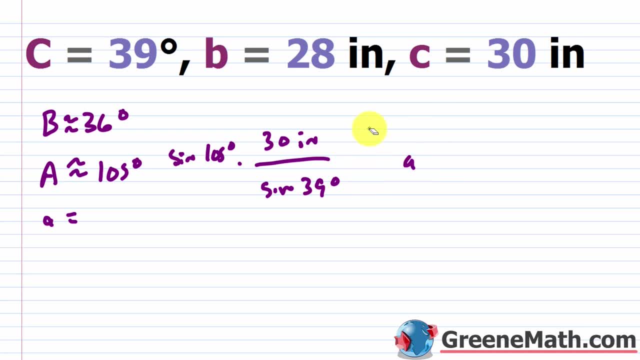 so you can show that here, if you want to, and say this is approximately a- okay, Most teachers will allow you to put equals there as well. And I'll go ahead and say this is about 46 inches. So let's say it's about 46 inches, okay. Now let me show you this sketch really quickly. 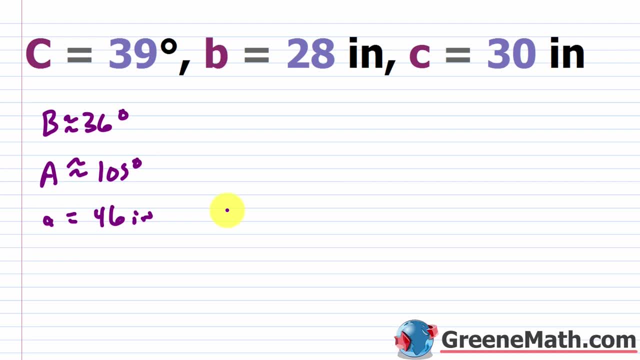 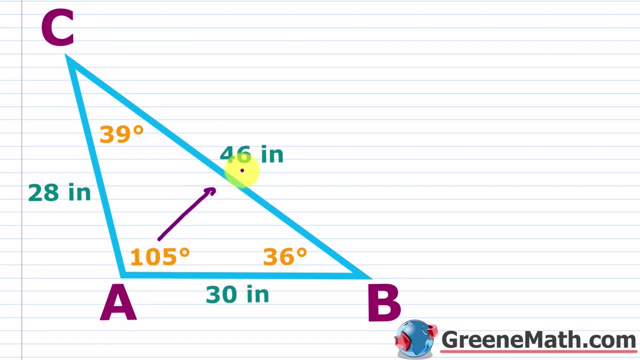 and then I'm going to come back and show you why there can't be two solutions, okay, How you can prove this. So let me show you the sketch I made. So here you have your angle a which is 105 degrees. Opposite of that, you have your side a which is 46 inches. Again, this is an approximation. 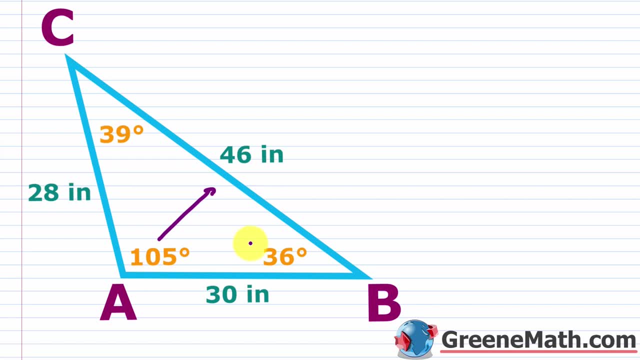 For b, it's 36 degrees Opposite of that, okay. over here you've got 28 inches. And then c is 39 degrees Opposite of that. you've got 30 inches, okay. So let's go back up. Let me show you why. 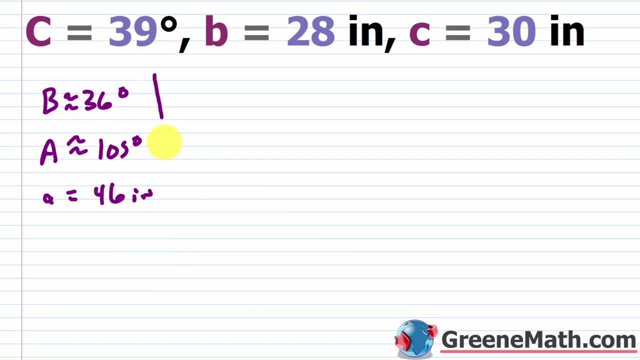 there can't be two solutions. We saw: let me just erase, or actually, let me just box this off. We got an angle measure here of 36 degrees for b- okay, Approximately, but let's just work with that. If we look in quadrant two and we think about: okay, what angle has a reference angle? 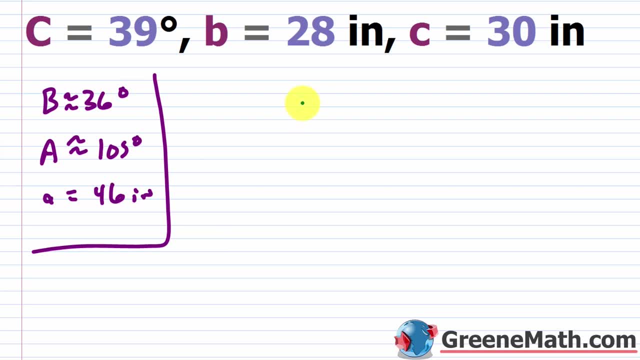 of 36 degrees. Again, we can't just say, okay, what angle has a reference angle of 36 degrees? Okay, we can't just say, okay, what angle has a reference angle of 36 degrees? And again, we talked about this earlier, you would take 180 degrees, you would subtract away 36 degrees. 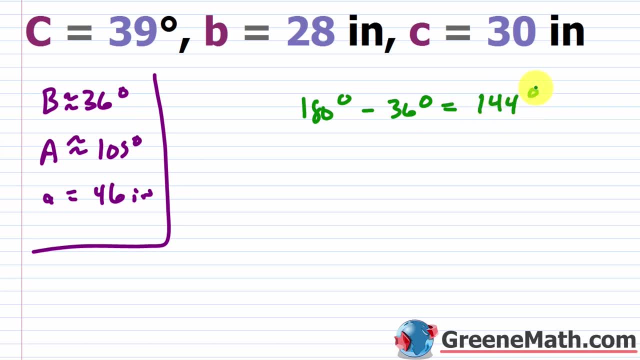 and that would give you what? That would give you 144 degrees, okay. So remember when you did that inverse sine operation. that's only going to give you something in quadrant one or four. okay, We're working with positive values here, so you're always going to get. 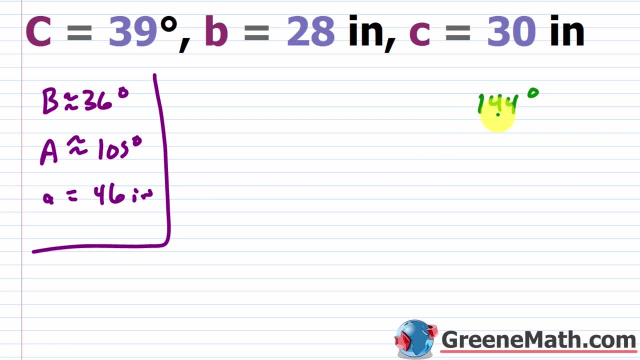 something in quadrant one. If you want to go into quadrant two and get something, okay, the something that has the same sine value, in this case 144 degrees- you've got to use that concept of a reference angle. The problem here is that if I say that b could also. 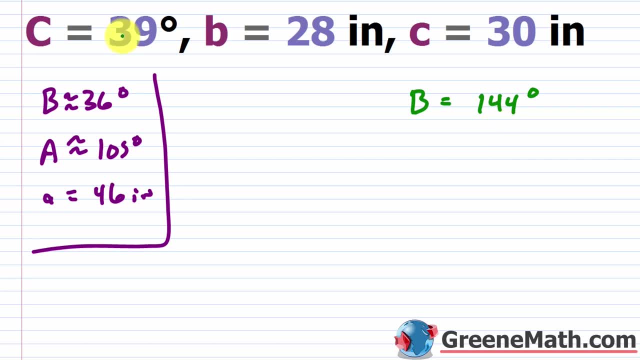 b equal to this, even if it was approximately. well, we're given that c, here is 39, right degrees. So 144 plus 39 is going to give me 183.. Remember the sum and let me make that better. 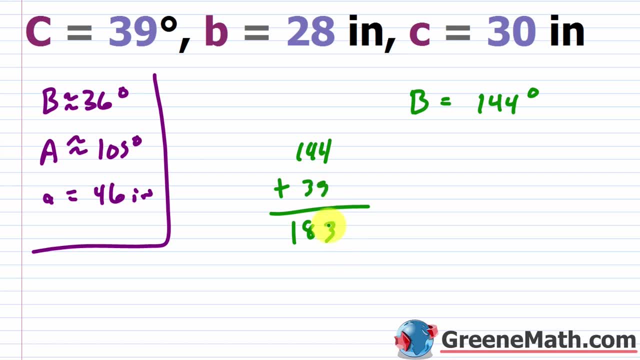 the sum of the three angles in a triangle is 180 degrees, So this is not possible. I can't have something that's 144 degrees because I'm going to go over. okay, So you can go ahead and exclude that right away. If you want to prove that to yourself, you can. But again, if you get an 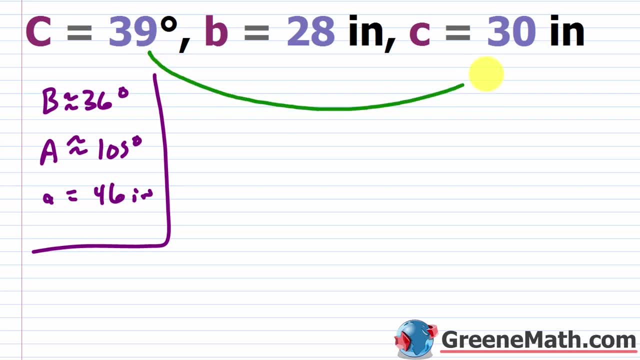 angle- in this case it was c, it's 39 degrees. And then the side opposite there, which is 30 inches, is bigger than this b that they're giving you. okay, the side in that position, which is 28 inches. you can go ahead and conclude that you're going to have exactly. 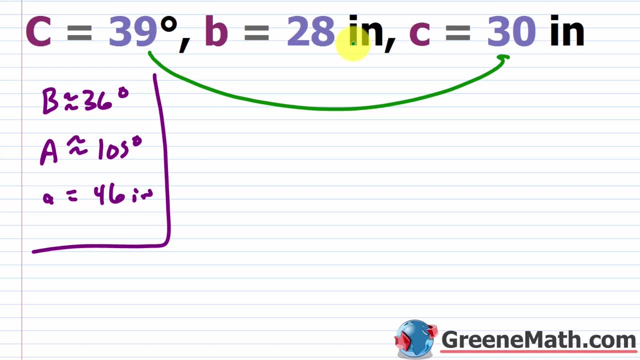 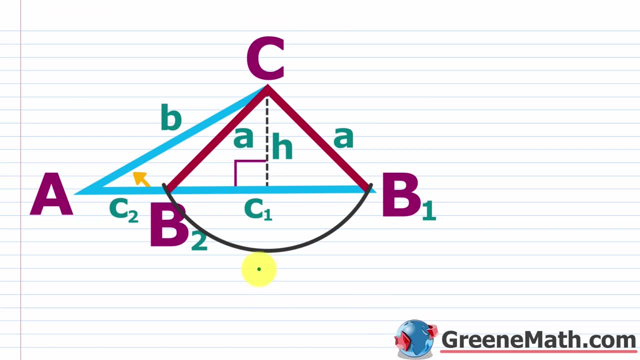 one triangle and it's not going to be a right triangle in this case. All right, let's go ahead and take a look at one final scenario with, given an acute angle and its side opposite. So you'll see this diagram or this image. here is pretty busy, a lot of stuff going on because we're 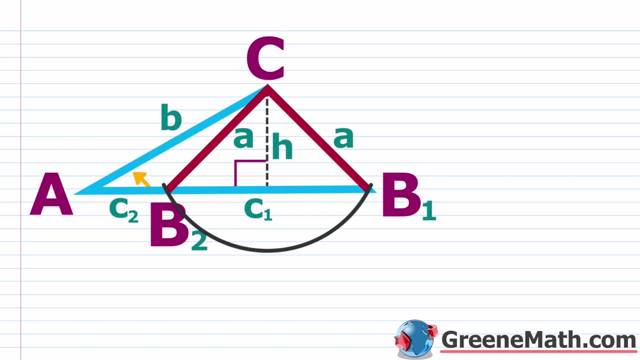 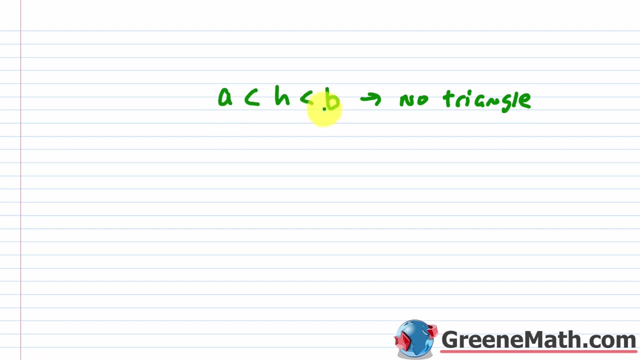 going to have two triangles here. So let me just quickly recap a few of the things that we've already seen. So we saw that if a was basically less than h and h was less than b, that there was no triangle, right? So there's no triangle in this particular case, But notice that a here is less than b. So 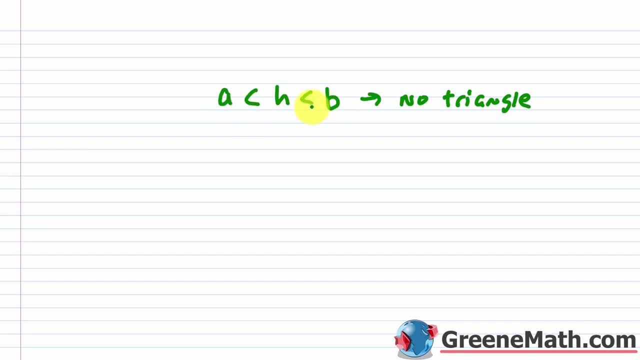 this is kind of one of the things where you have to really be careful about what you're doing, because if you see a is less than b, you could have no triangle. or if we're going to see in a second, you could have two triangles. Then we saw that if a was equal to h, okay and you could. 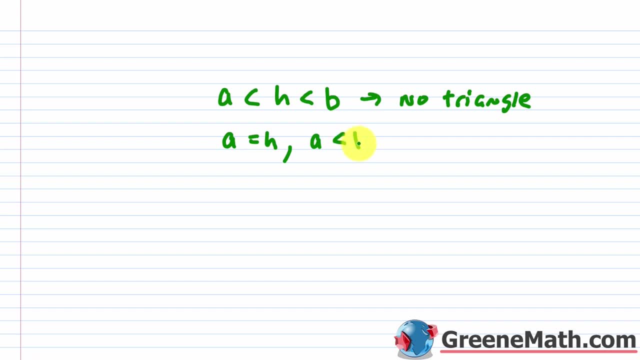 say a or h, whatever you want to do, if a basically is less than b, then you would have a right triangle and you would just have one, obviously. So one right triangle, okay. Then we saw that if a was greater than or equal to b, you would basically have: 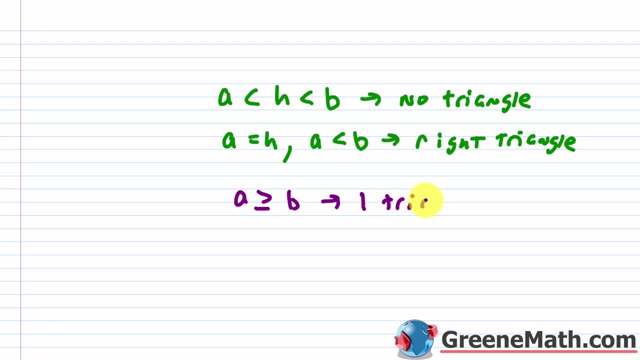 and let me not put a comma there- you would basically have one triangle. So one solution, one triangle. Here. what you're going to see is that a is greater than h and it's less than b, So when this happens, you're going to have exactly two triangles, okay. So some students don't like. 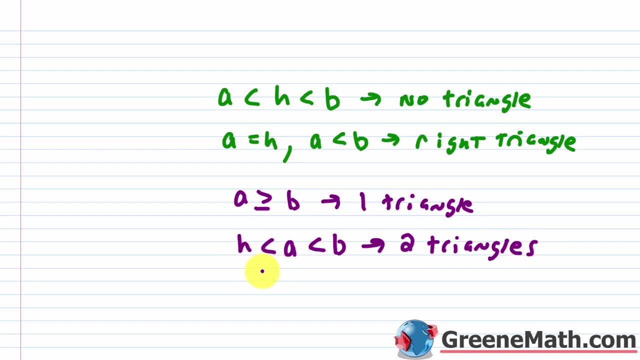 to check things this way. They don't like to involve h and you don't have to right, You can use your law of signs. So if you're using the law of signs with this guy, when you try to find the sign of the angle b, it's going to be greater than 1, okay. So that's how you know you have no. 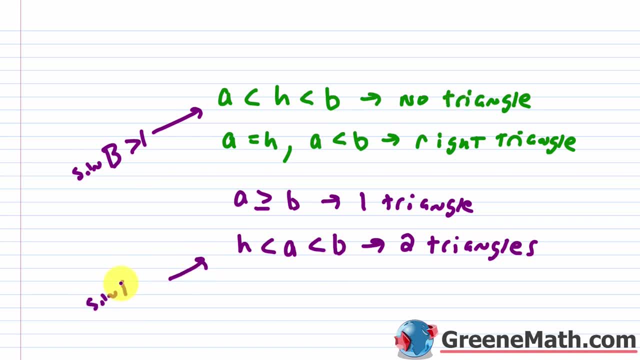 triangle Here, when you try to find the sign of b, it's going to be greater than 0. So you can say it's going to be greater than 0 and less than 1.. So this guy is going to give you your two triangles. 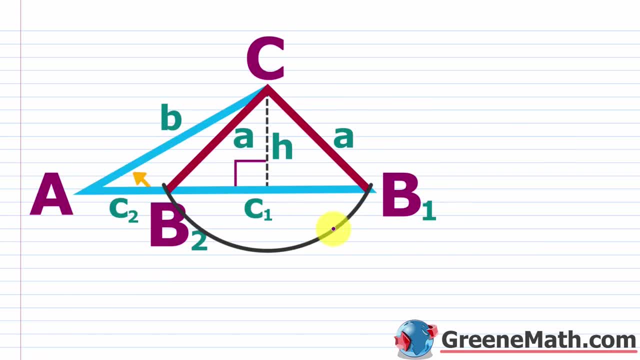 This guy gives you your no triangle, okay, So it's important to understand. When we return here. let me go ahead and write this again. So a is greater than h and less than b. okay, When we return here, a is going to be the same in each case. It's just how it's drawn, okay, So you'll. 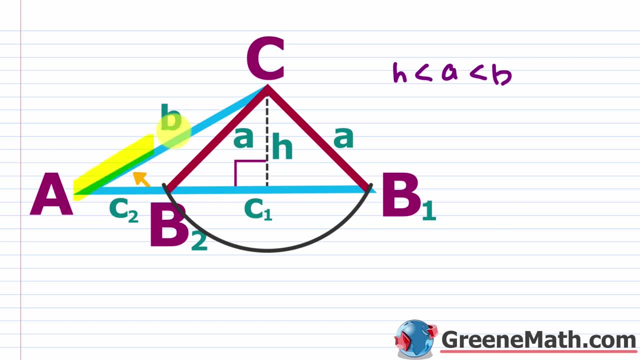 see this in your book, this little swing here. So basically the first way you could draw a triangle this way, okay, So basically you'd have this b sub 1 here. That's your angle b, You have your angle c here And then down here I put c sub 1.. Most books don't even put a c down. 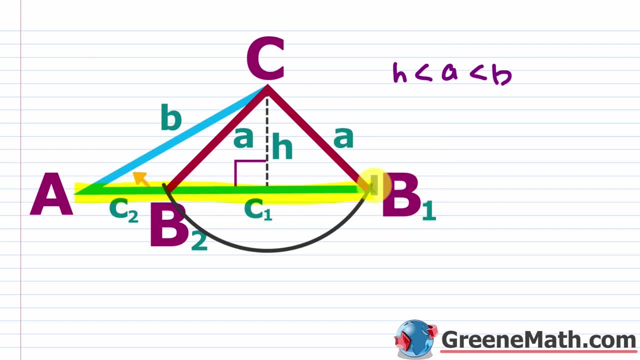 there. But basically, c sub 1 would be from a to b sub 1, like that. okay, So the length of the entire thing, That would be your side c. Now if we swing it this way, okay, and we draw this a different way, 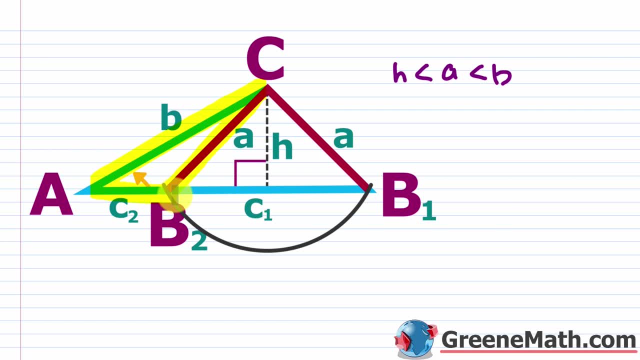 it's the same, But now my triangle is going to look like that. okay, basically, And so when you think about c sub 2, now it's just going to be this short piece here, right? So that's my. 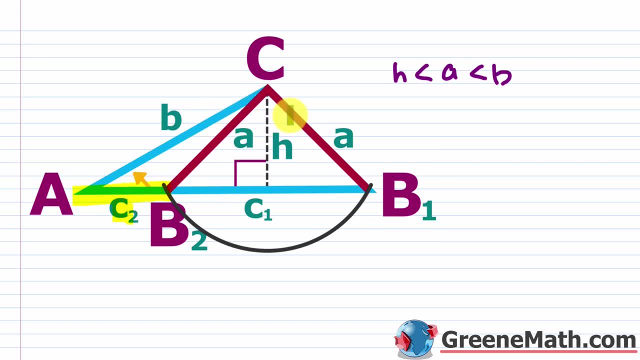 side c. So the angle c changed, okay, from basically here to just a smaller version, okay, And the angle b changes as well. So you're going to see the angle b change, the angle c change and the side c change when you look at these guys and draw up two triangles. 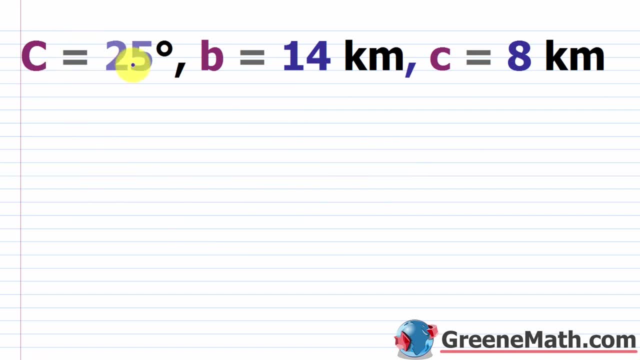 Let's go ahead and look at an example here. So we have: c is equal to 25 degrees, We have b equals 14 kilometers and c equals 8 kilometers. So again, when I think about this, I have the angle and it's. 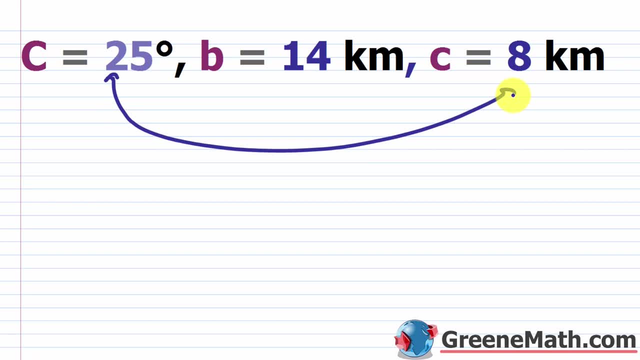 opposite. okay, Don't worry about the letters, It's completely irrelevant. okay, Don't get hung up on that. If I want to find h again, I'm using that same formula. Take this guy, okay. So this measure here that's not involved in the angle and it's opposite, multiply it by the sine of the. 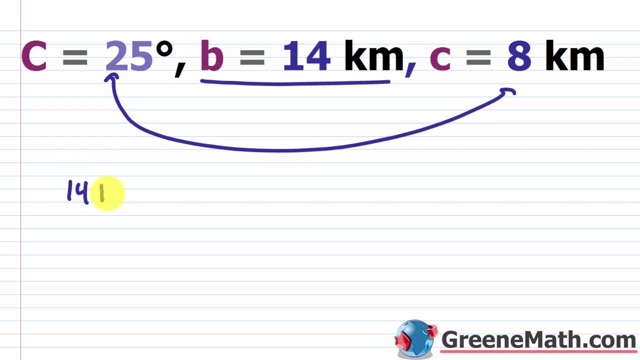 angle you're given. It's all you're doing. So I'm going to take 14 kilometers, multiply it by the sine of 25 degrees and this is going to be equal to h. okay, And I like my variable to be on the left. 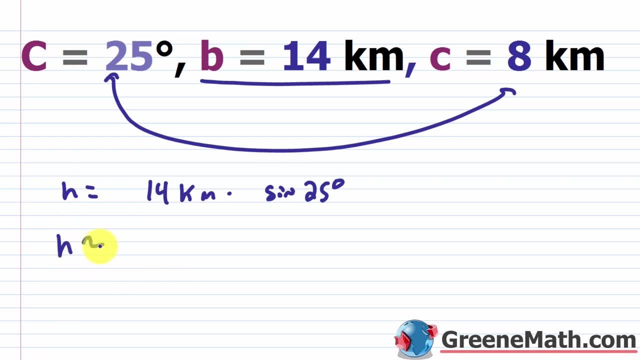 so let's just go ahead and put it like this: So h equals this. We'll say h is approximately. let's go ahead and say 5.9 kilometers. okay, So if I think about this, is this guy less than this? 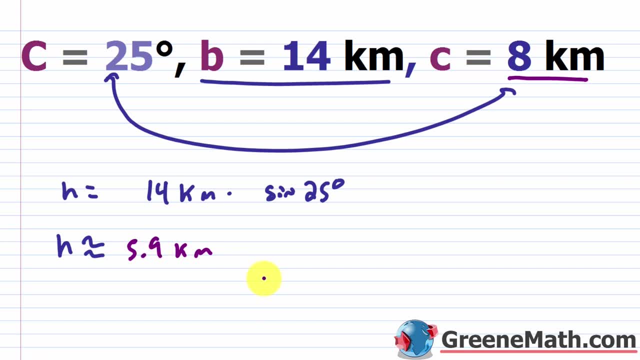 okay, and greater than this. Yes, right, If I line this up, I would say: 5.9 kilometers is less than 8 kilometers. okay, which is less than 14 kilometers. So I am in a scenario where I have two triangles. okay, That proves that. Now, again, if you just looked at this piece, 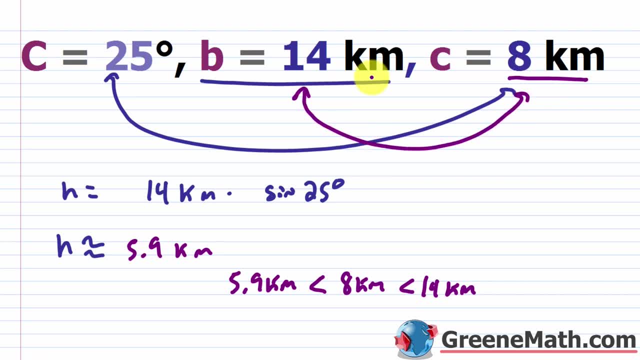 of information and this piece of information, you're going to see that this guy is less than 14 kilometers. okay, That proves that. Now, again, if you just looked at this piece of information and this piece of information, you can only conclude that you either have two triangles or no triangles. okay, So, 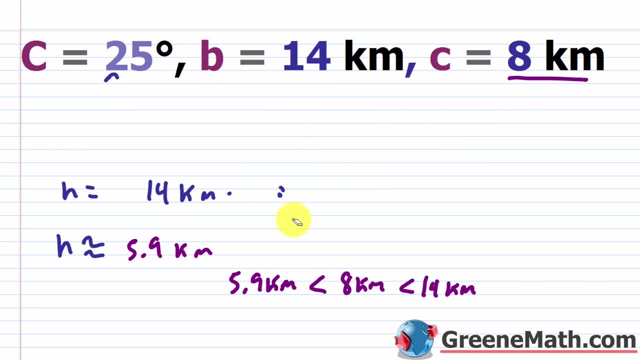 you'd have to use the law of sines to get further into that. So let's go ahead and do that right now so we can start solving this guy. We know we're going to have two, okay, So I'm going to first. 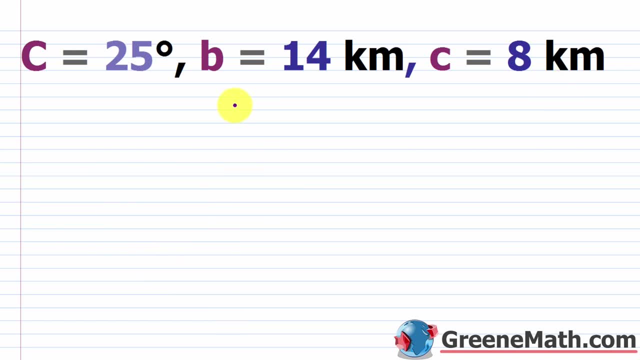 start by finding my angle b. okay, So how do I do that? Again, I would say that the sine of c- okay, so the sine of 25 degrees over c, which is 8 kilometers then, basically, is equal to the sine of b. 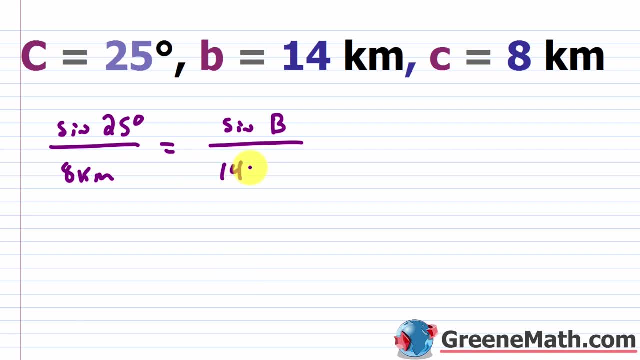 over. okay, I'll go ahead and say this: 14 kilometers here. Now I know I'm going to multiply both sides by 14 kilometers, so let me slide this down a little bit and let me do this in a different ink. So I'll say 14 kilometers. We know that this is going to 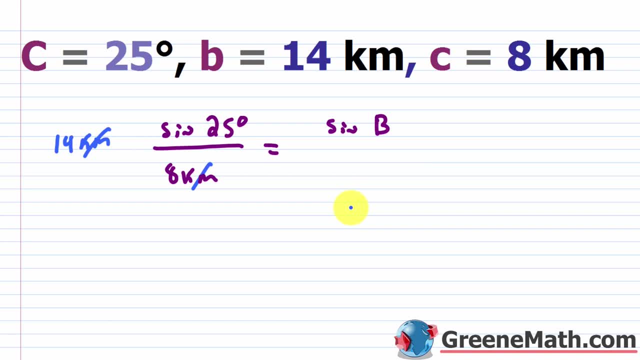 cancel here and let me just erase it from here. So what would this give us? We get about 0.739,. let's just go ahead and say 6.. So I'll say the sine of b is approximately 0.7396, okay. 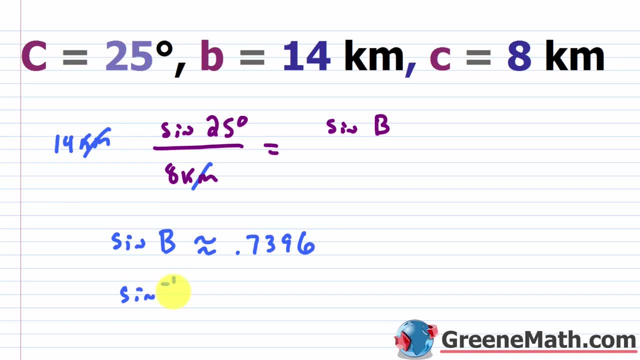 So you want to use your inverse sine function, so I'll say sine inverse of this guy right here, so 0.7396.. Again, if you wanted to wrap this guy right here, okay, inside the parentheses when you're doing sine inverse, that's fine too. okay, This is going to be more accurate Now if I do. 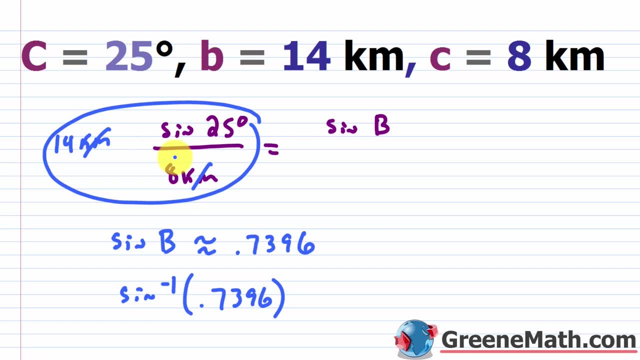 this. I'm going to get about 47.7 degrees. So let me erase all this and I'll say b, okay. b and I'm going to put sub 1 is about I put equals, so let me put approximately 47.7 degrees okay. 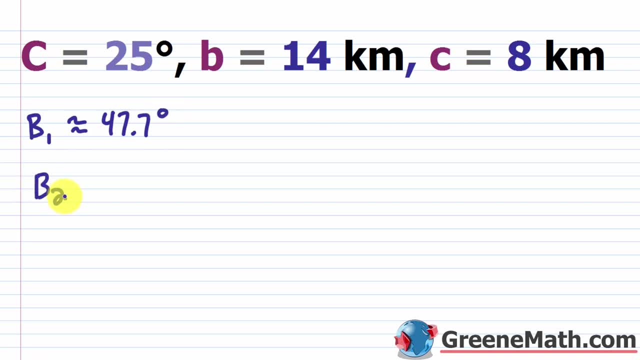 How do I get b sub 2?? Remember we talked about this earlier when we said we would use the concept of a reference angle. All we'd have to do is go into quadrant 2 and say, okay, well, 180 degrees. 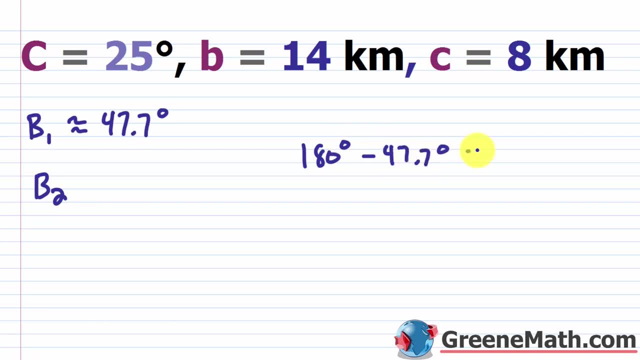 minus this reference angle, 47.7 degrees, would give me 132.3, okay degrees. So I'll say this is approximately 132.3 degrees. okay, Now I'm going to separate these two, I'm just going to. 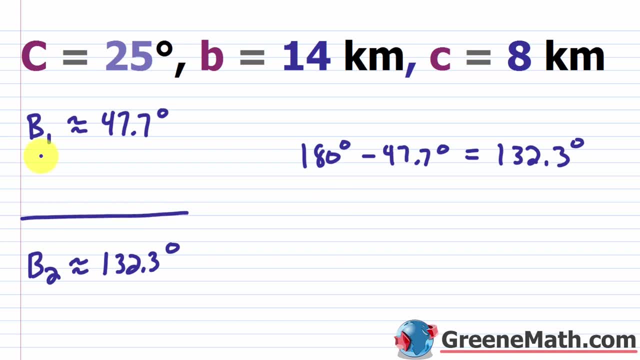 put you know, maybe a border here or something like that, because we do need to find everything. a and you could put sub 1, and you want to put lowercase a here, sub 1, right? So this is all for. 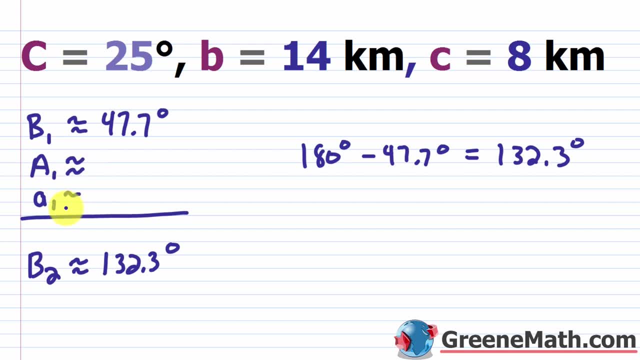 the first time. okay, So I'm going to put approximately and approximately, and let's just erase this real quick, okay. So another thing here too, and I didn't do this. basically, you know this is going to work because, again, when you add this, so 132.3 degrees plus this, 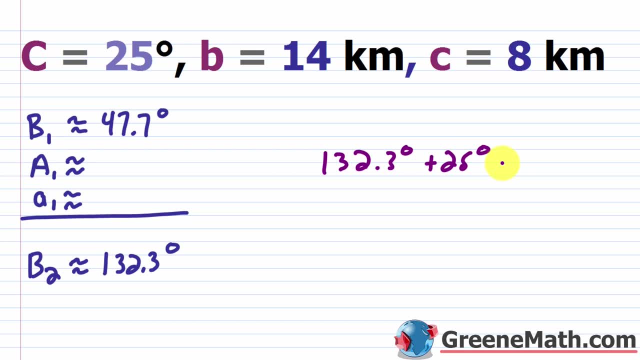 25 degrees here. this is not going to be greater than 180 degrees. We saw earlier in the lesson. we tried to add these guys together. We got 183 degrees, so it was greater than 180 degrees, so it didn't work. Here you have room for another angle, because this is going to be 157.3 degrees. 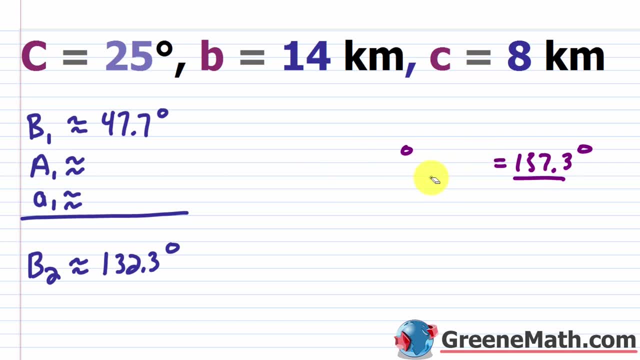 okay. So you see here for sure, this is going to work and you're going to have two triangles, okay, So let's erase this. Let me also add down here: I'll put a sub 2, okay, And I'll put: 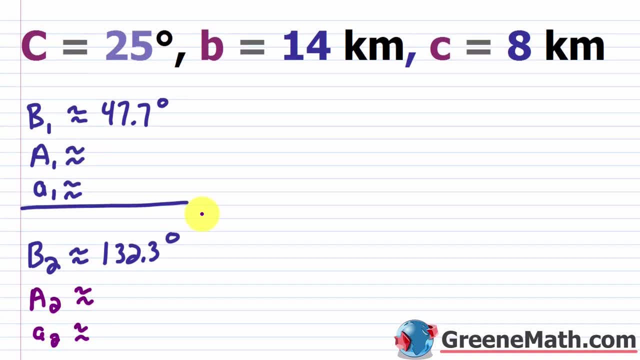 lowercase a sub 2 like this. So let's work on this first one here. So if I want a sub 1, all I need to do is go 180 degrees minus 25 degrees minus 47.7 degrees. So this is going to give me, we'd say, 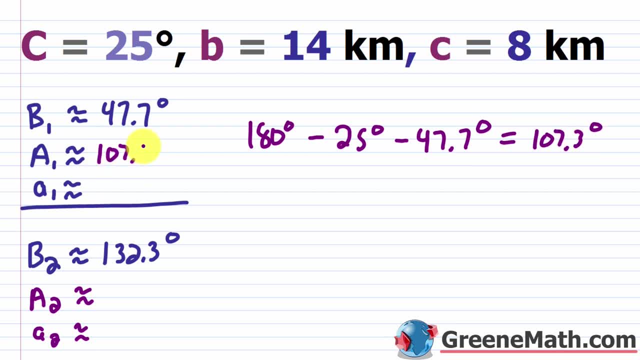 107.3 degrees. So this is going to be 107.3 degrees. So let's erase this. And again we're going to use our law of sines, So I'll go ahead and say that I have 8 kilometers over the sine. 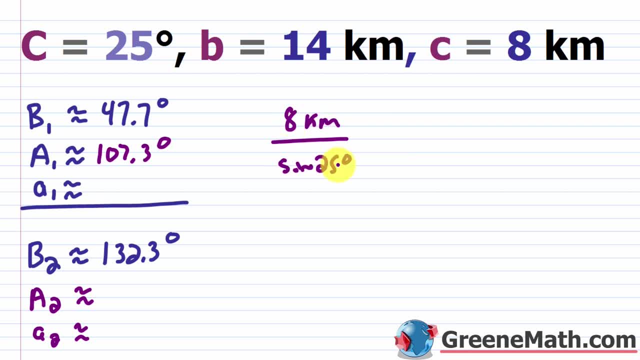 of 25 degrees. So this is basically c over the sine of c. I'm going to multiply this by. in this case, I would have the sine of 107.3 degrees. okay, This will be equal to a. Again, if I did a. 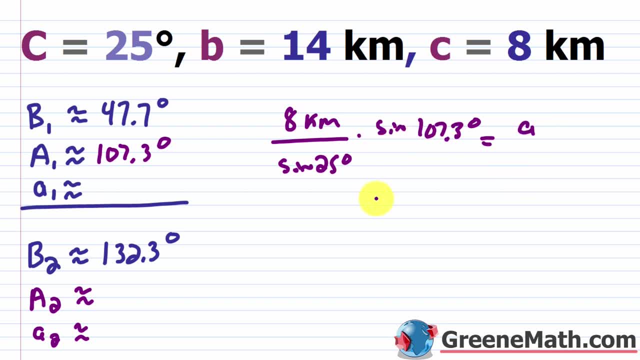 over the sine of a, I would end up multiplying both sides. So I'm going to multiply both sides by this. That's how I got that, okay? So if you punch this up on a calculator, we'll say: this is about 18.1, and this is going to be in terms of kilometers, So we'll say 18.1 kilometers, okay. 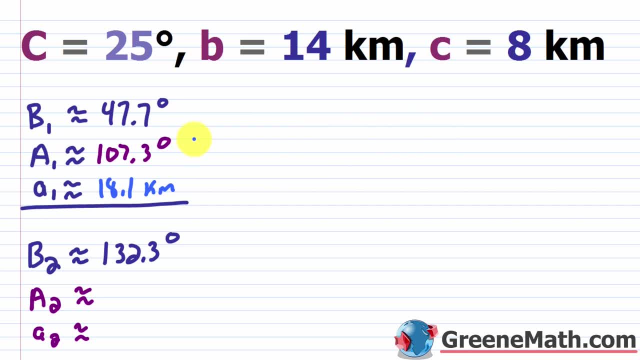 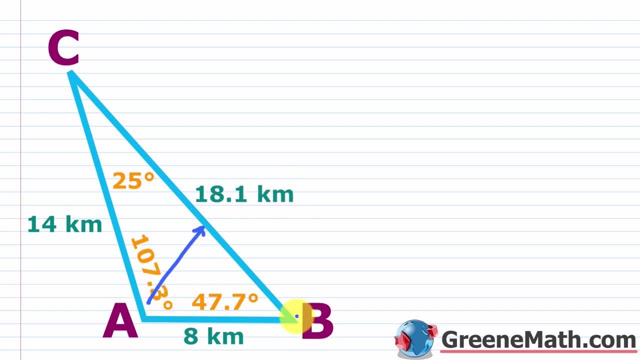 Let's erase this And I'll quickly show you the sketch of this guy. So you see here, your angle a is 107.3 degrees. Opposite of that, I've got 18.1 kilometers. Your angle b here is 47.7 degrees. 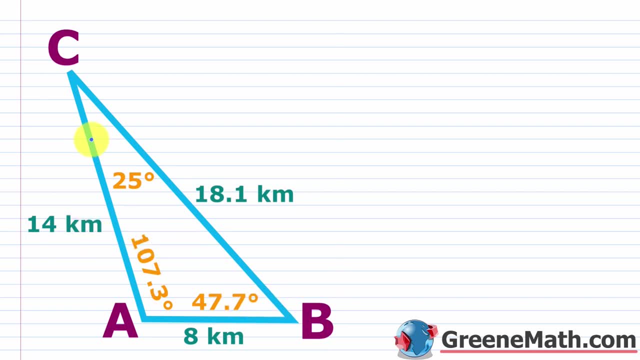 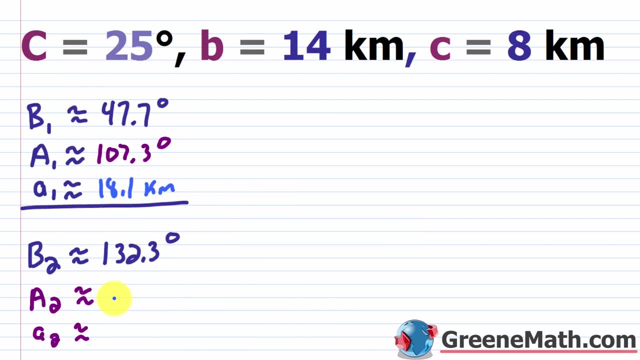 Opposite of that, I've got 14 kilometers. And then your angle c here is 25 degrees. Opposite of that is 8 kilometers. okay, So let's go ahead and look at the other guy And again we're going to solve things in a similar way. So now for a sub 2, I'm going to have 180 degrees. 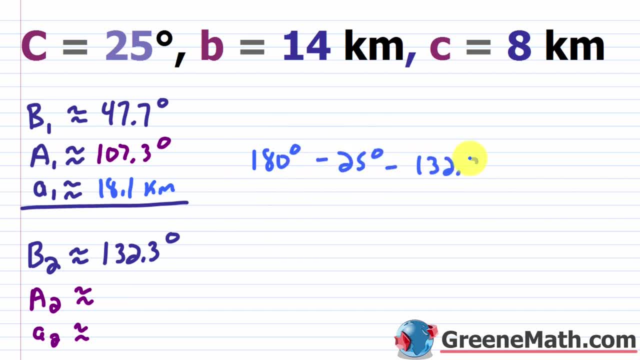 minus 25 degrees, minus now 132.3 degrees. So this equals 22.7 degrees. okay, Let's put 22.7 degrees in like that, And now I just need a sub 2.. So again, I'm just going to do the same thing. 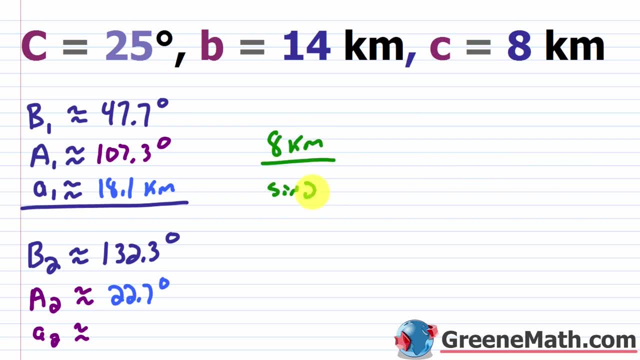 So I'm going to go 8 kilometers over the sine of 25 degrees times- In this case, I'm going to do the sine of this guy. So 22.7 degrees, okay, And this is going to be equal to a. So let's go ahead and punch this up on a calculator And you're going to get an a. 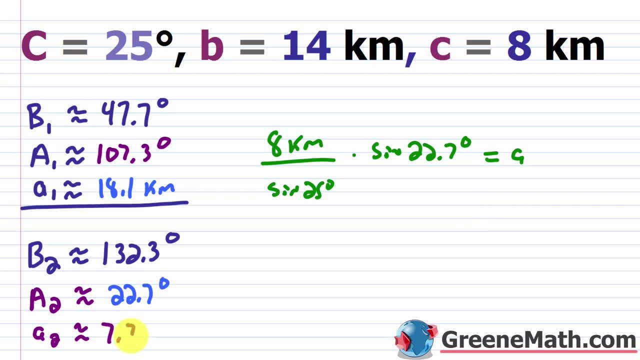 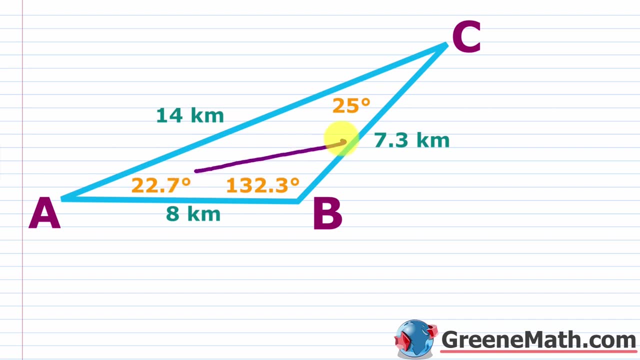 is approximately 7.3.. And this is in terms of kilometers. So 7.3 kilometers like this. So let's erase this Again. I've drawn this triangle for us. So if we look at our sketch here, we have our angle a, which is 22.7 degrees. Then, opposite of that, I'm going to do the same. 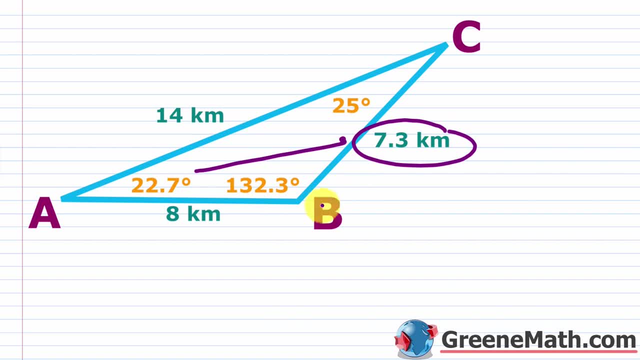 thing. We have this 7.3 kilometers. Then we have our angle b, which is 132.3 degrees. Opposite of that, we have our 14 kilometers. Then we have our angle c, which is 25 degrees Opposite of that. 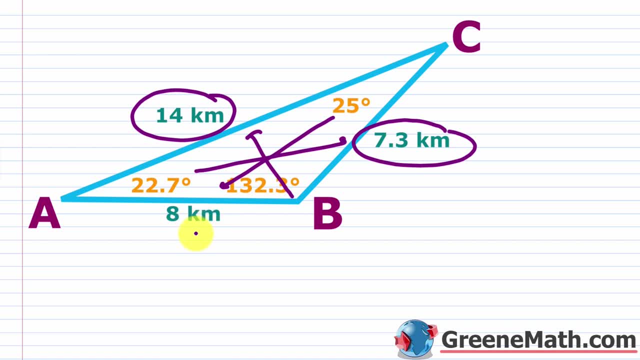 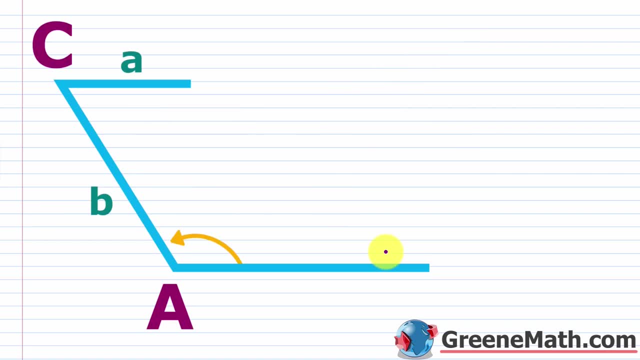 we have our 8 kilometers. So, based on the information given, we can see that we can draw two different triangles. All right, so let's move on to the final two scenarios. These are pretty easy overall. This is when the angle you're given is now an obtuse angle. 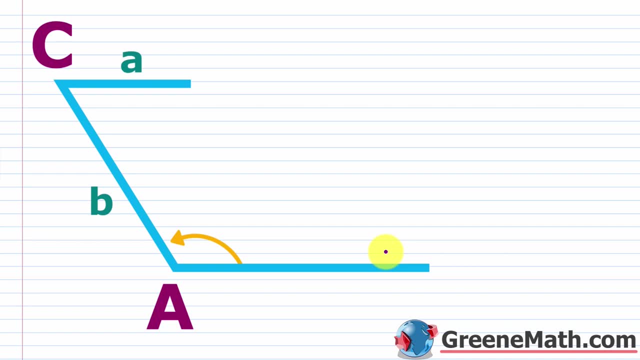 So basically, you just have two situations that deal with this. The first one is, let's say, you have some angle a. it's obtuse and you're given that And you're given the side opposite of that. so this a here If a is less than or equal to b. 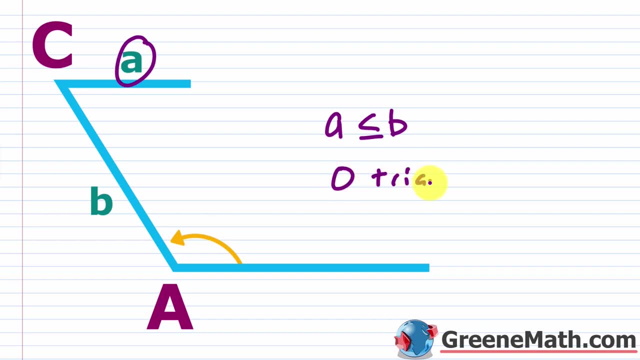 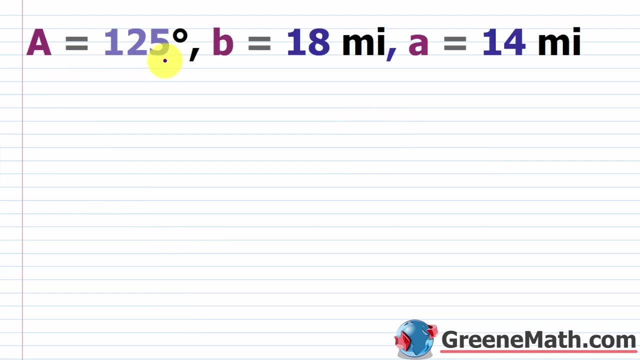 so if a is less than or equal to b, then you'll have zero triangles. So zero triangles, or you could say no triangle will exist. Let's look at an example. So here we have: a is 125 degrees, b is 18 miles and a is 14 miles. So again, this a right here is opposite of this. 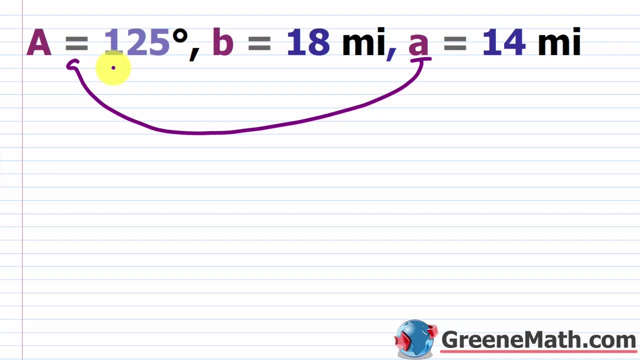 angle a here, which is 125 degrees. By rule, every angle in a triangle is going to be the largest angle, So therefore it should be opposite the largest side, and it's not right. This right here, this 14 miles, this 14 miles. okay. 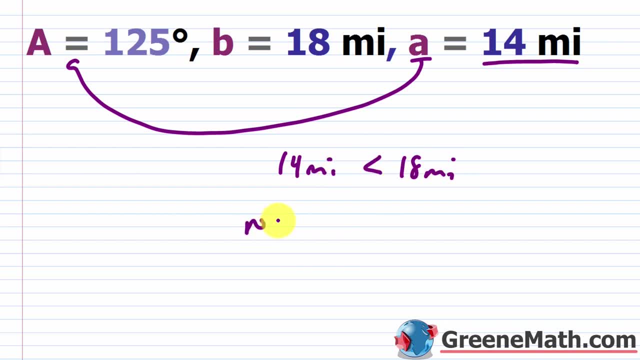 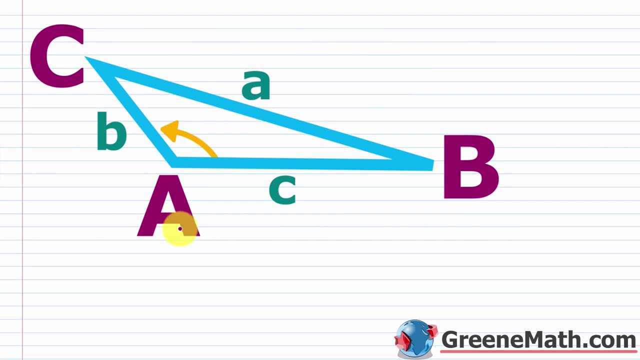 is less than this: 18 miles. so there's no triangle right. No triangle, no triangle exists, exists- I guess I could clean that up a little bit, so let's make that better. So exists. For the final scenario, we're given some angle a. again it's an obtuse angle. 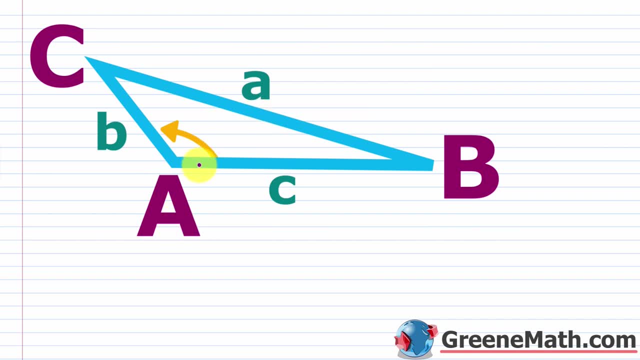 and we're given the side opposite, okay, And then we can basically say: this side opposite, a, in this case, is greater than b. So if a is greater than b here, so if this is greater than this, we'll have exactly one triangle. So let's look at an example. So here we have: a is 114 degrees. 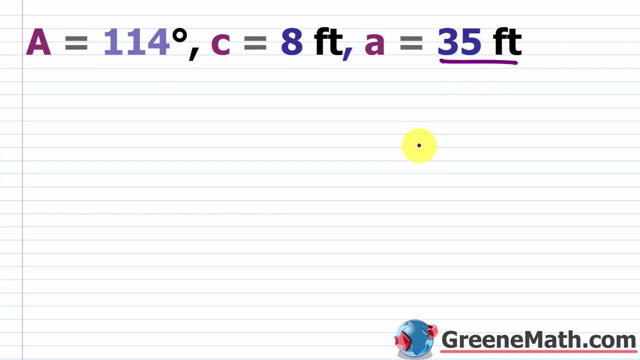 c is 8 feet and a is 35 feet. So clearly this right here, okay, which is opposite of this right here- is larger than this other guy you've got. So what I would do here is start by finding my c. So I would do the sine of c is equal to- let's go ahead and say- the sine of 114 degrees. 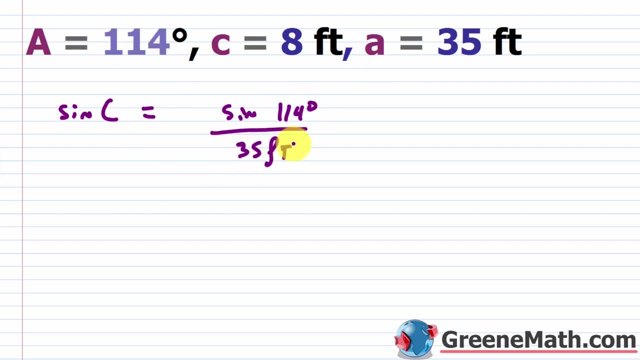 so the sine of a over a itself, which is 35 feet times, it's going to be c, which is 8 feet. okay, So remember, you divide sine of c by 8 feet and you multiply both sides by 8 feet. 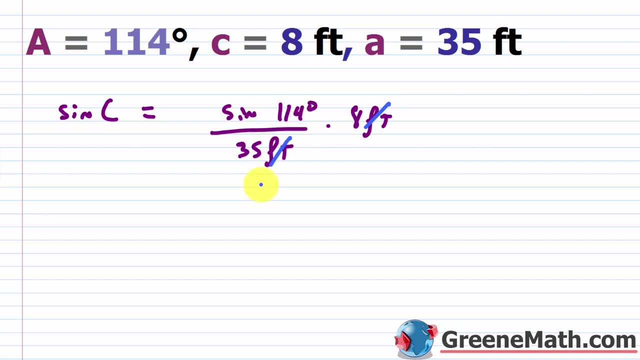 so that's how we set this up, So we know that this is going to cancel with this, and so basically, what you'd have is about 0.20, let's say 8,, 8,, okay. So let's say: 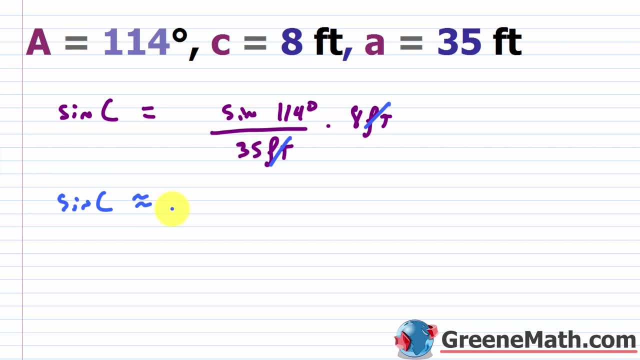 the sine of c is approximately, I'm going to say, 0.2088,. okay, So we're going to do the inverse sine. so sine inverse of this guy, 0.2088,. this is going to be equal to, let's say, about 12.05,. 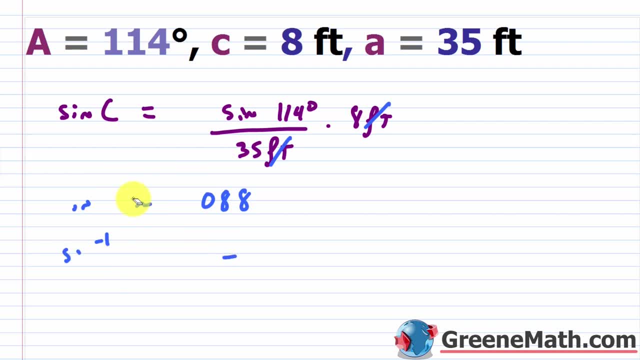 so maybe we'll go 12.1.. So let's say that c, just erase this and put c is approximately 12.1 degrees. okay, Erase this, all right. so now let's go ahead and find my b. so this is approximately what. 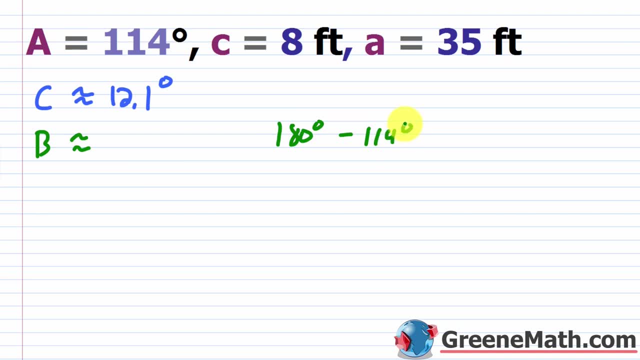 Well, I'm just going to do 180 degrees minus 114 degrees, minus 12.1 degrees, and this is going to be equal to, let's say, 53.9, okay degrees. So we'll say this is: 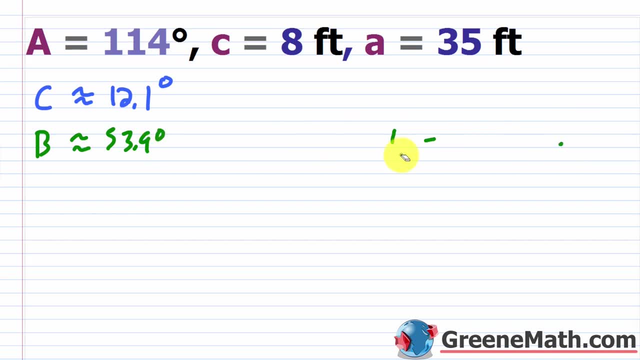 approximately 53.9 degrees. okay, So we have that. and, lastly, we just need this lowercase b or this side measure. so let's go ahead and put this as approximately what, Again, I'm going to use the sine of c. so let's go ahead and put this as approximately what, Again, I'm going to use. 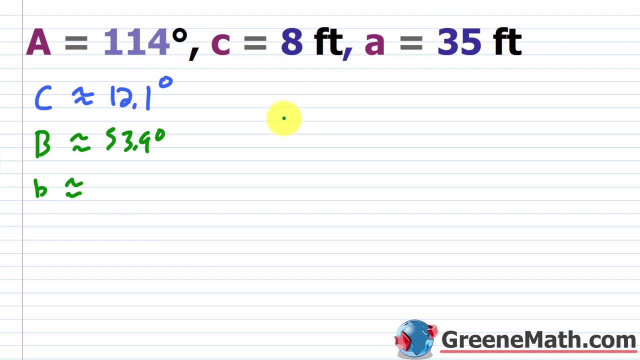 the information I'm given. so I'm given a and then a here. so I'm going to say, since I want lowercase b, I'll say b is equal to, or put approximately whatever you want to do. I'm going to say it's going to be this: 35 feet, okay, So over we'll do the sine of 114 degrees, so a over. 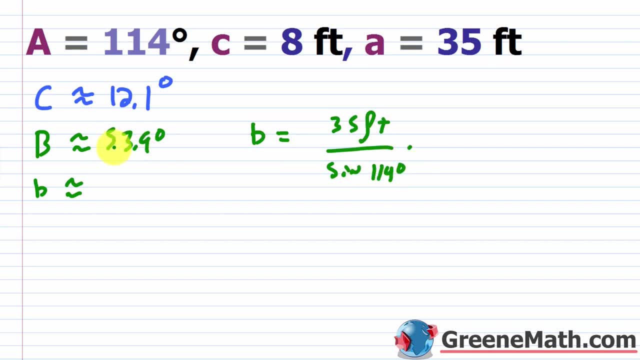 the sine of a and I'm going to multiply this by the sine of this b here, so the sine of 53.9 degrees. Again, we would have had b over the sine of b. so I just multiplied both sides by the sine. 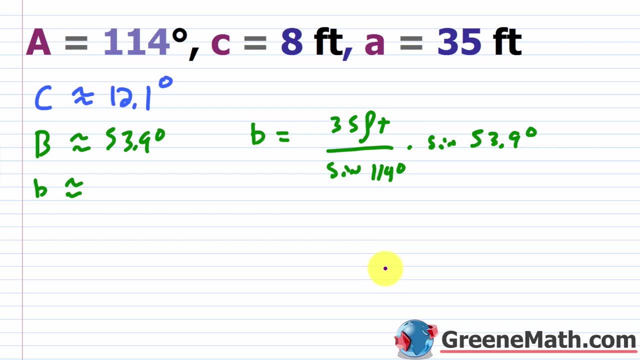 of b. so that's how I got that set up, okay. So basically, what I'm going to have here is, let's say, about 31 feet, okay. So let's say approximately 31 feet, okay. All right, so we've solved this. 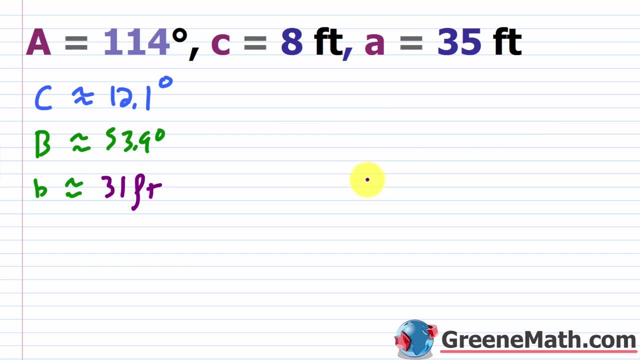 triangle When you get the obtuse situation. it's much easier When you're dealing with an acute angle and the opposite side okay. that's when you really have to dig into the details and really think: If you get an obtuse angle and it's opposite side, that's pretty easy, right? You're? 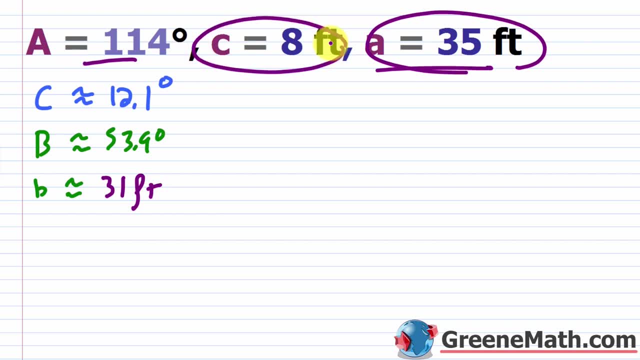 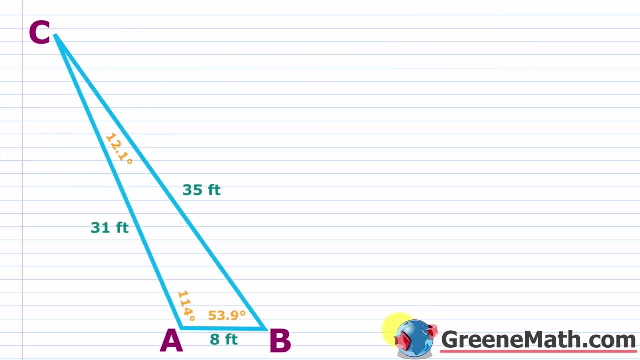 larger than this one right here that they gave me. If it is, you have one solution. If it's not meaning they're equal or it's less, then there's no solution. okay, No triangle. So let's go down and look at a little sketch here. So I have: angle a is 114 degrees and again opposite of that. 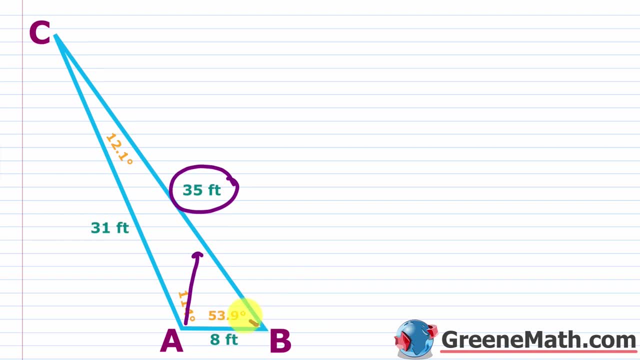 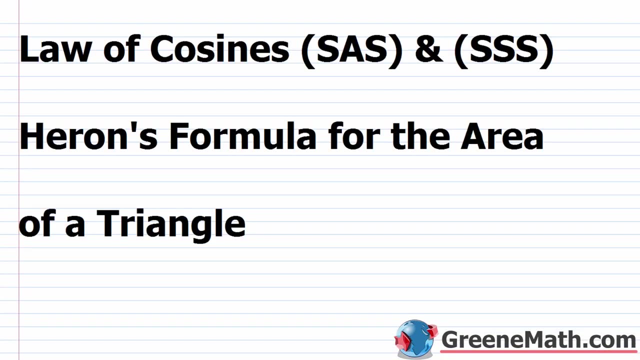 you have the 35 feet. Angle b is 53.9 degrees. opposite of that, you have 31 feet. Angle c is 12.1 degrees. opposite of that, you have 8 feet. In this lesson we want to talk about the law of. 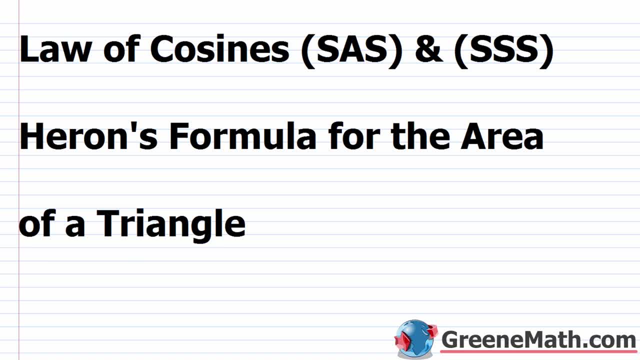 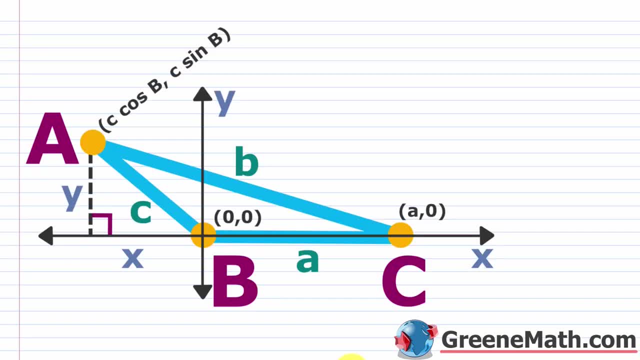 cosines with the side angle side and the side angle side. So let's go ahead and look at the side side side, and also we'll look at Heron's formula for the area of a triangle. All right, so over the course of the last two lessons, we've been learning about how to solve these. 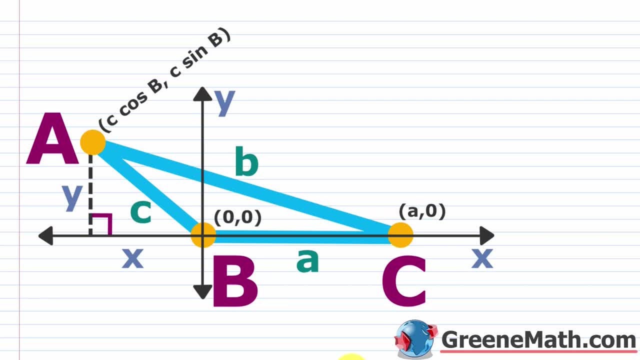 oblique triangles using the law of sines. So we saw the easy case with the two angles and the side given angle, side angle or side angle angle, okay. And then we saw the harder case, the ambiguous case of the law of sines, where we had to think about things right. This is where 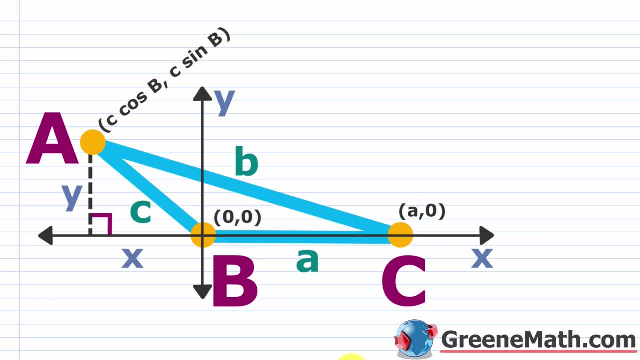 we had two sides and a non-included angle, so side side angle. Now we're going to look at something that is a little bit different, right? So we're going to have side angle side, so two sides and an included angle, and then also side side side, right. So all. 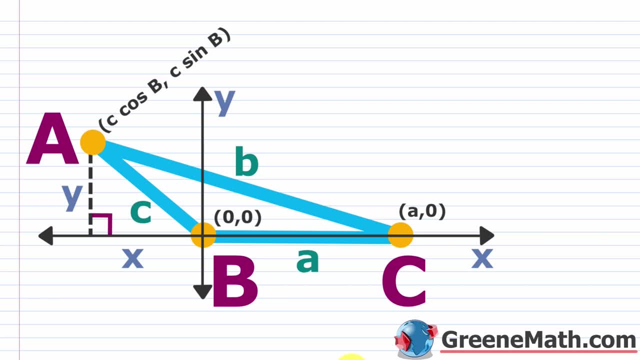 three sides, no angles. When these two cases present themselves, we're going to be using the law of cosines now okay, And we're going to say that a unique triangle can be determined So we don't have to go through all this stuff that we saw with the ambiguous case of the law of sines. 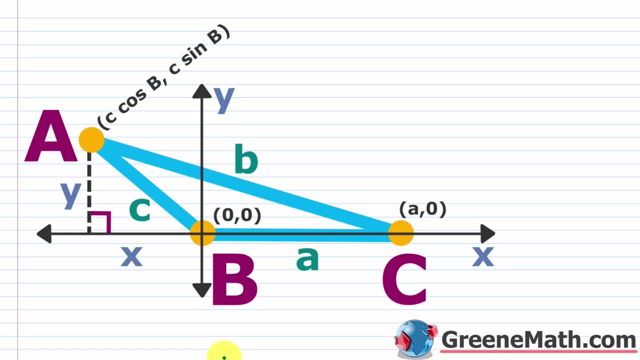 All right, before we get going on some problems, I want to give you some insight in terms of where it comes from. I'm not going to go through deriving each one, because there's going to be three of them, but I'm going to show you one of them and you can get the other ones on your own. 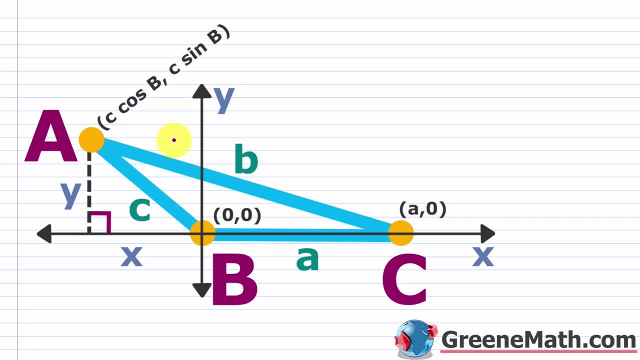 if you want. Now, some of you might not find this very interesting. Some of you might find it extremely boring. Just skip ahead to the problems, if that's you okay. So the first thing is you'll notice that we have this triangle here and it's an oblique triangle and it's named ABC, okay. 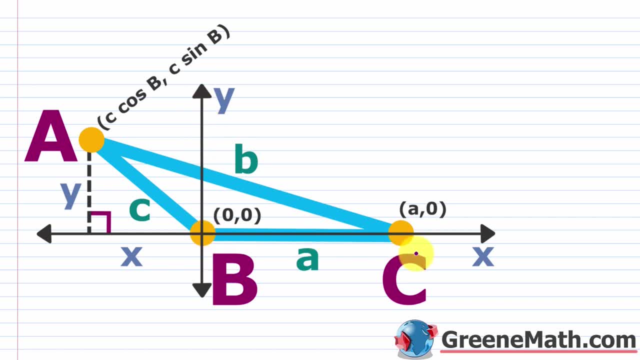 Typical. Now you'll notice that we put this guy on the coordinate plane, okay, Where B basically is at the origin, right. So we have this 0 comma 0.. You'll see, for C, you have this A comma 0.. So 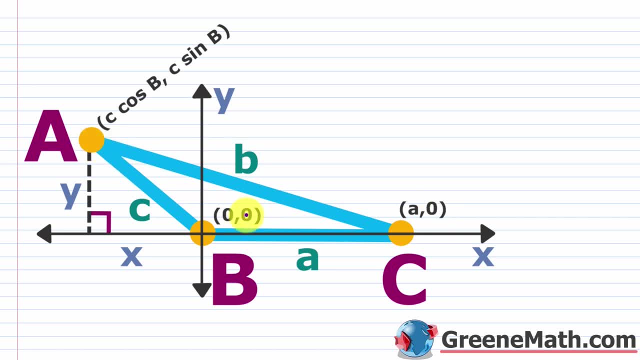 where does this come from? Well, opposite of angle A, you have side A right Labeled with this lowercase a right. So this is a length. You can think about this as the line segment BC. okay, right here. okay, Well, basically, this has a length of A, so the X coordinate, there would be A. 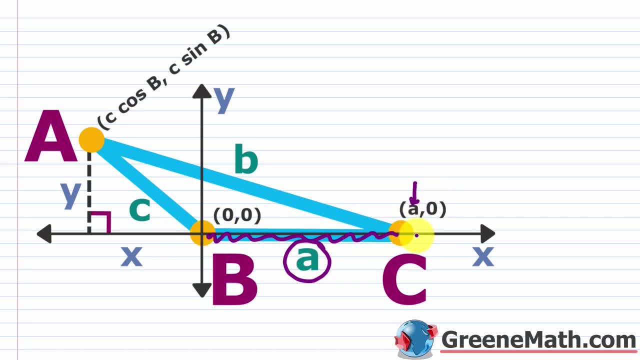 The Y coordinate would be 0, because you're still on the X axis, right. So that's where we get the A comma 0 there. okay, Now up here, this one might be a little bit more difficult to understand. but basically, to get this guy right here and this guy right here, you could start off by calling: 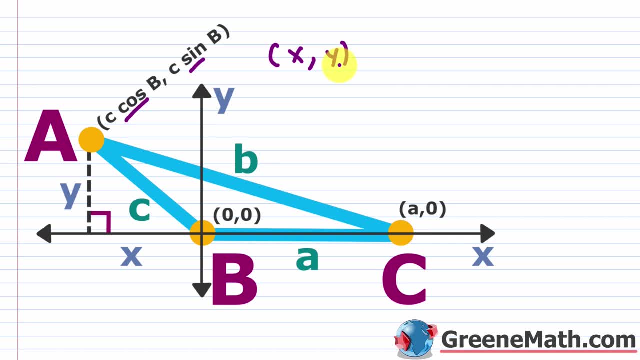 them X, comma, Y, okay, Just start with that generically. Then what you would do is you would take the sine of this angle B, okay. So how would we do that? Remember, this is an obtuse angle here. so what you do is you'd form this right triangle here, okay, Like this, and you'd say: 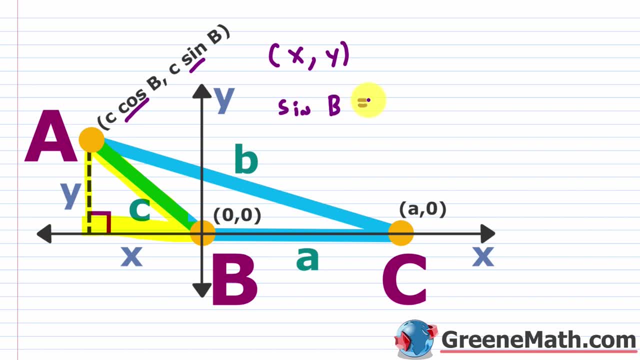 okay, the sine of B is going to be equal to what. It's going to be equal to the opposite, which, in this case, is going to be Y over the hypotenuse, which in this case is C. so Y over C, okay, And then let's go ahead and do the. 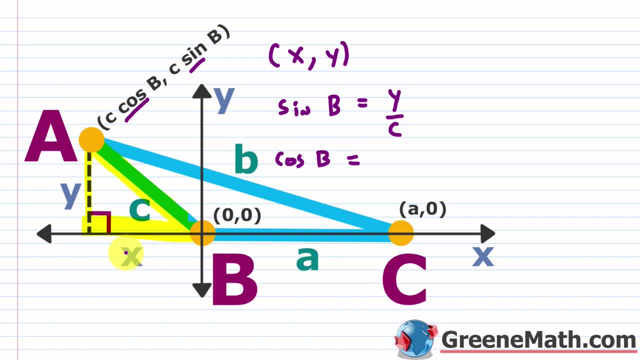 cosine of this angle B. also, Here you have the adjacent over the hypotenuse, so this is X over C. okay, So so far, so good. Now, where does this come from this C times cosine of B and C times sine of? 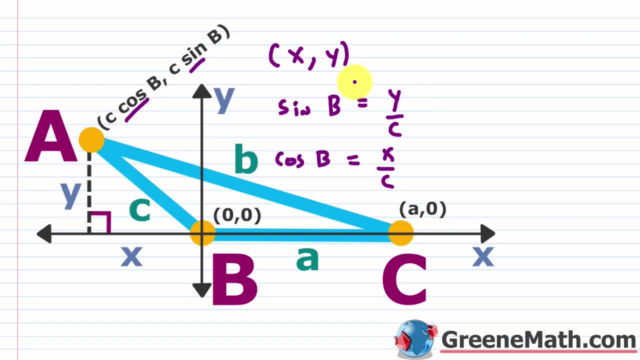 B: Well, basically you're just going to solve for Y and then solve for X and then plug in in each case. okay, That's all you're doing. So I'm going to multiply here both sides by C, so by C, by C. 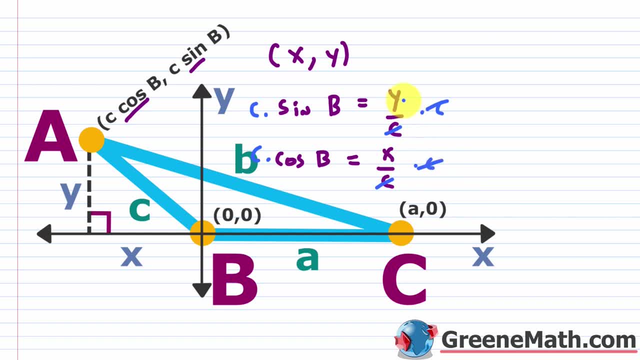 and basically over here this is going to cancel, cancel. So Y equals C times the sine of B, and here you see, C times the sine of B. okay, And here X equals C times the cosine of B, and again C times the cosine of B. So you're just taking what? 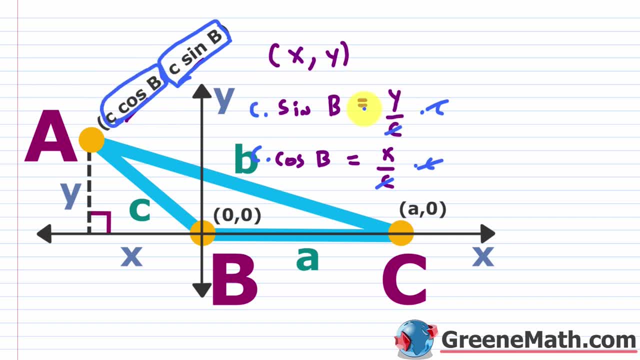 X is and you're plugging it in there. okay, You're taking what Y is or what Y is equal to and you're plugging it in there. So that's where all this stuff comes from. So let me erase. 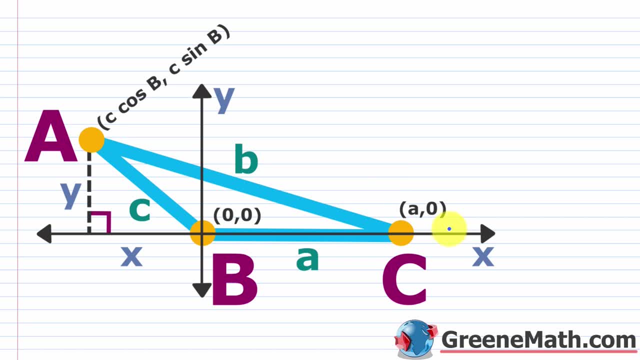 everything. and now let's talk about a formula to find basically the length of this guy right here. So this would be using the distance formula. We know how to do this from, say, basic algebra, but again I'm going to call this side here: B right, Lowercase B. 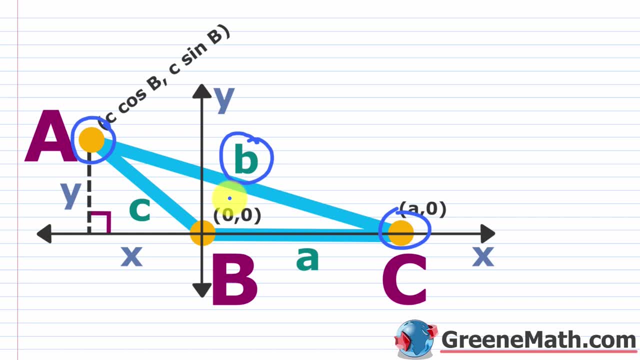 because it's opposite of angle B. So how would we do this with the distance formula? We would say what? Let's just write it here real quick. So we have D. the distance between these two points on the coordinate plane is equal to the square root of. you have your X sub 2 minus your X sub 1. 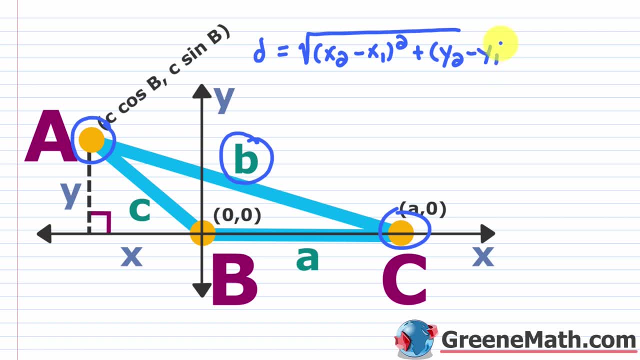 quantity squared plus your Y sub 2, minus your Y sub 1 quantity squared. Okay, so from here now D with B, because the distance from here to here it has a name, lowercase B, So let's put that in. 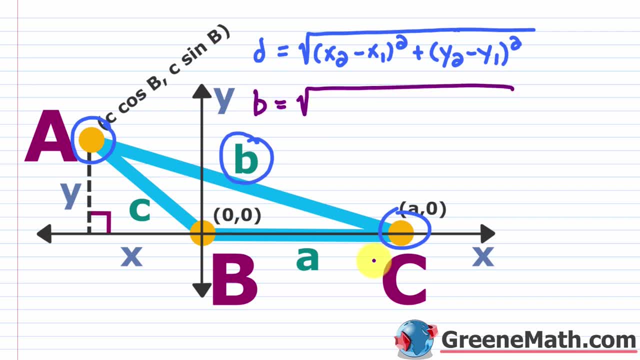 there. okay, And this is the square root of again. it doesn't matter how you pick these points. I'm going to label this guy right here as X sub 2, Y sub 2, and I'll label this one as X sub 1, Y sub 1,. 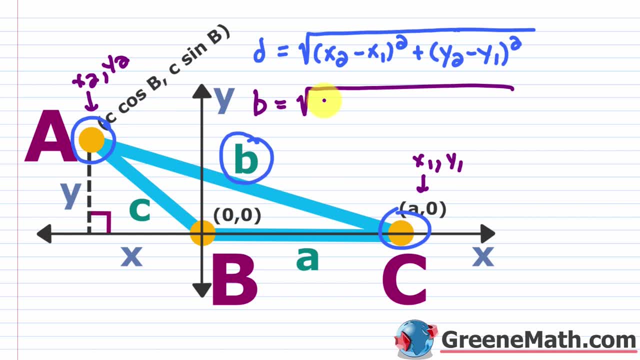 just to make it easy. So I'm going to plug in C times cosine of B, So C times the cosine of B, and then basically minus A. this quantity will be squared and then plus- we're going to do this- C times sine of B, So C times sine of B, and then you would do minus zero. I mean, I can put that in. 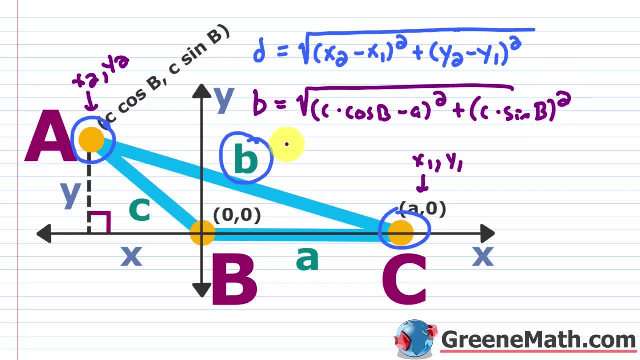 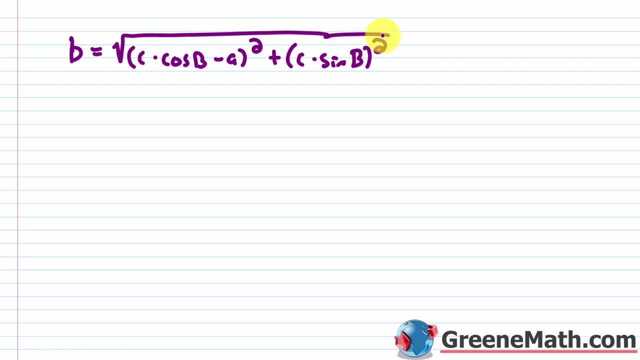 there, but it doesn't really do anything. So I'm just going to close this and square, okay. So let me copy this real quick and let's paste this here, so we have a lot of room to work, okay, So basically, the first thing you would do here, I mean you could square everything inside first- 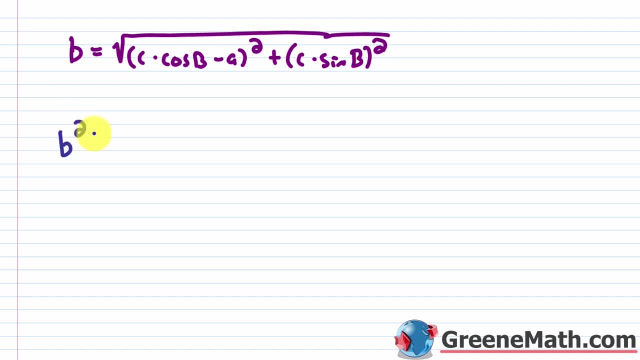 but I'm just going to square both sides and I'm going to say: B squared is equal to remove the square root symbol. so you're going to have C times cosine of B minus A- this quantity squared plus. I'm going to have C times the sine of B- this quantity squared. 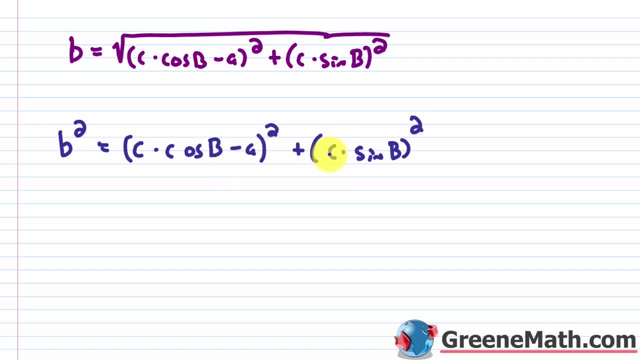 okay. So basically, what we want to do here is just expand everything, right? So this one right here. this is just multiplication, So you can just apply your exponent in each case, right? So this will be C squared times sine squared B. okay, But for this one right here, you have two terms. 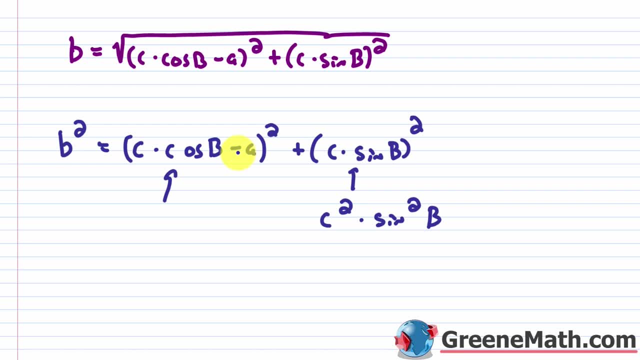 right. So you have to expand that or basically foil it out right? In this case it's a special product formula, So I'm going to have this as C squared okay, First guy squared times, cosine squared B. okay, So this whole thing is squared right C. 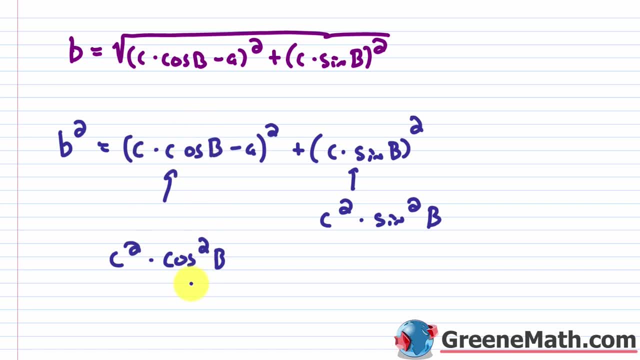 squared cosine, squared B. right, Because cosine of B is squared. okay. Then you'd have minus two times this guy times this guy. So two times C, times cosine of B, then times A. okay, If you want to write AC there, we can kind of rearrange that, make that a little bit cleaner, And then 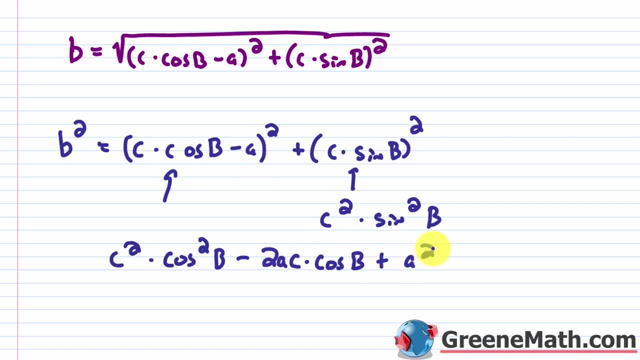 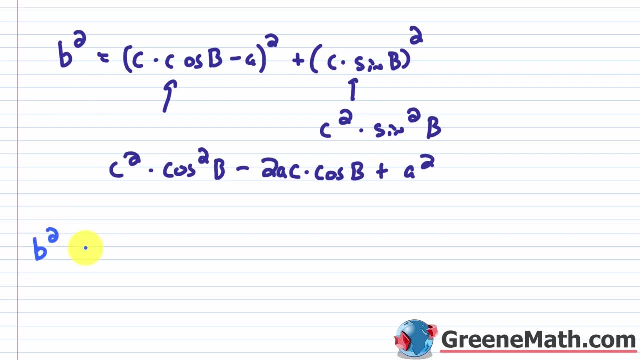 after that you'd have plus the last guy, which is A squared okay. So let me put all this together and let's go ahead and say: don't forget this B out here. So I'm going to say this is B squared okay, Is equal to. 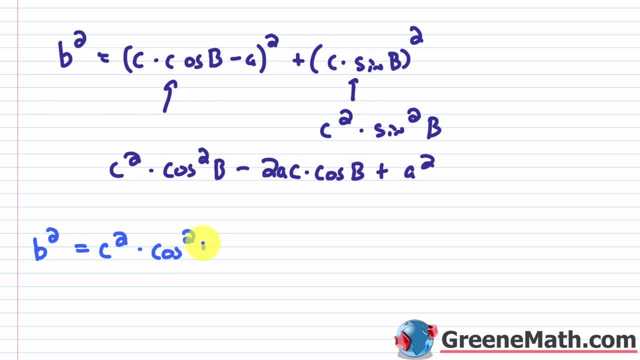 this is going to be C squared times, the cosine squared of B and then minus. we have two AC times the cosine of B and then plus A squared, and then don't forget about this one. So then plus C squared times sine squared B. okay, So I can erase this at this point. I'm just doing that for. 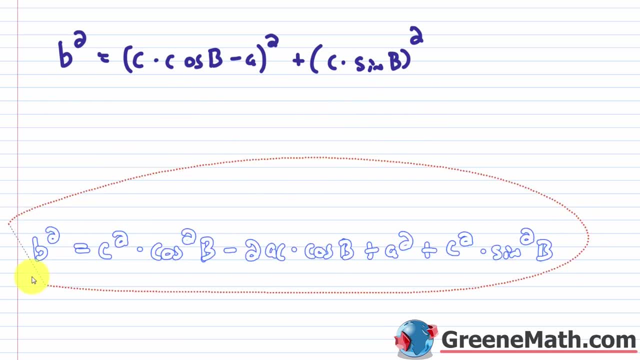 kind of side work or scratch work. So I don't want that to confuse you, So I'm just going to get rid of it. Okay, let's move this up here Now. one thing that might not be completely obvious, but you remember from probably earlier in the 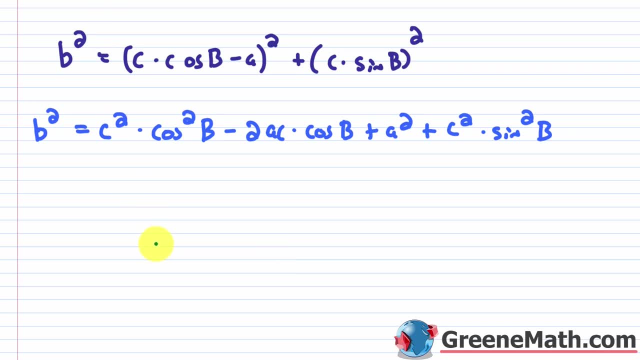 course, we saw something where we said: sine squared theta plus cosine squared theta equals one. You have a cosine squared B and you have a sine squared B here, okay. So if I can get those two together, they're going to be equal to one, okay. So this is what we're going to do. Let's. 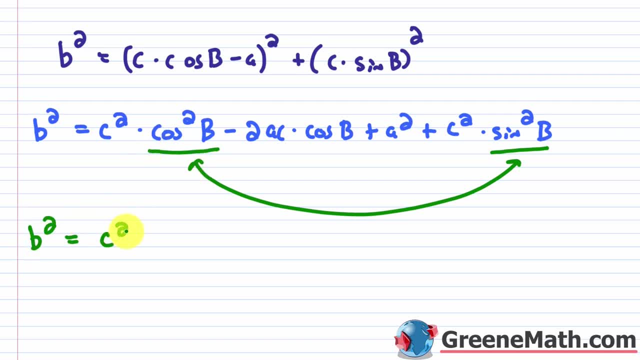 go ahead and say we have B squared is equal to. I'm going to go: C squared times cosine squared B, okay, And then I have this as a term here. this is a term, and then this whole thing is a term, So I'm going to put this over here. 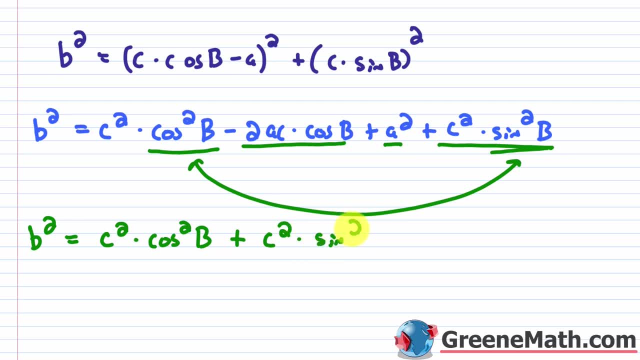 So plus C squared times sine squared B. okay, And then what didn't I use? I didn't use this and I didn't use this, So let me put those after. So let me go plus A squared and then minus two. 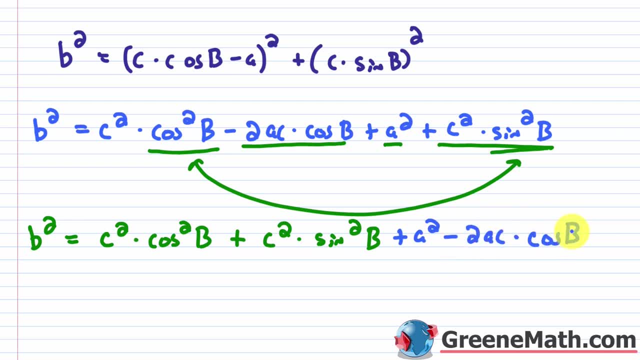 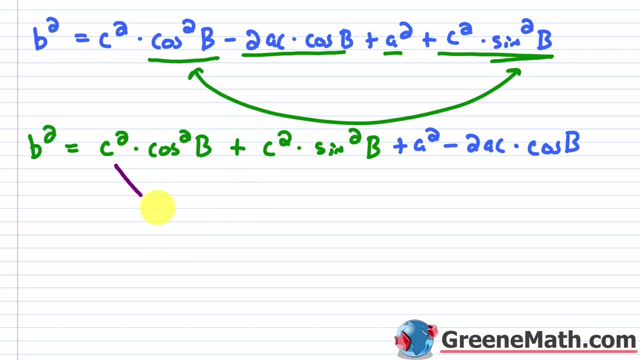 AC times, the cosine of B. okay, So some of you will see where I'm going with this. Others will be lost, and that's fine. I'll show you right now. Basically, what I'm going to do here is factor out. 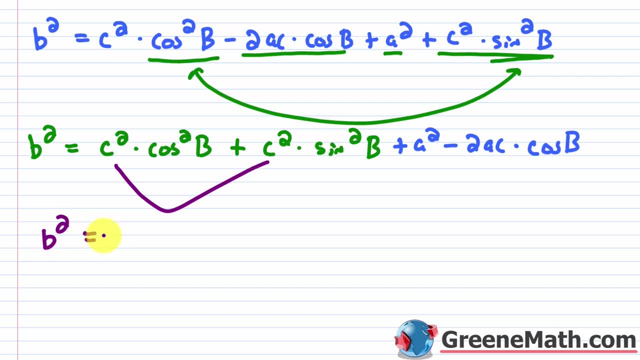 the C squared. Okay, So I'm going to have the B squared is equal to. we'll have this C squared out here and then inside you'll have cosine squared B plus sine squared B. okay, So that's taken care of. 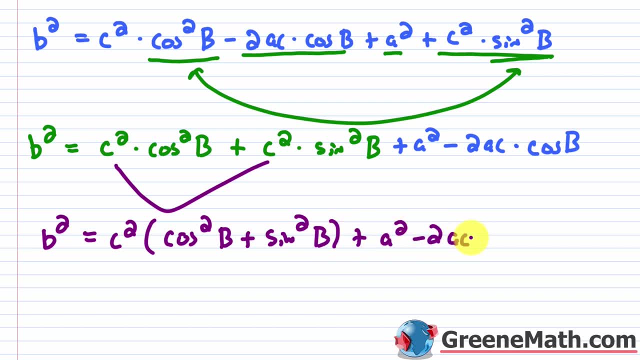 And then plus, you have your A squared minus two AC times the cosine of B. okay, So this right here we know, is equal to one right By definition. So you can erase this and just put a one in there, or just erase it all together, because you don't need it anymore. 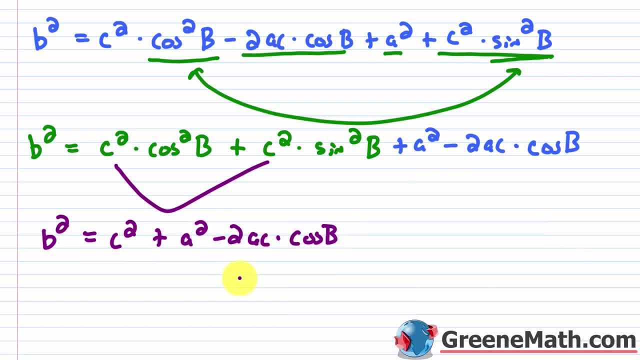 So let's move this down here. okay, Slide this down here and basically you're done. So this is the law of cosine. So B squared is equal to C squared, then plus A squared, then minus two AC multiplied by the cosine of B. Now in your book it's going to be rearranged. 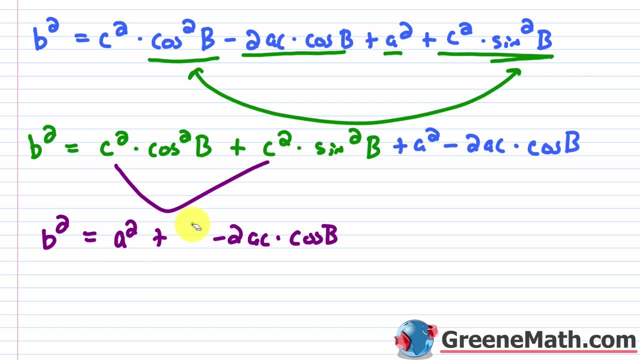 They'll put A squared here first, okay, And they'll put C squared here in the second position, But again, because this is just addition here, it wouldn't matter, okay, But this is how it's going to be listed in your book. so I want to be consistent. So where would this be useful? 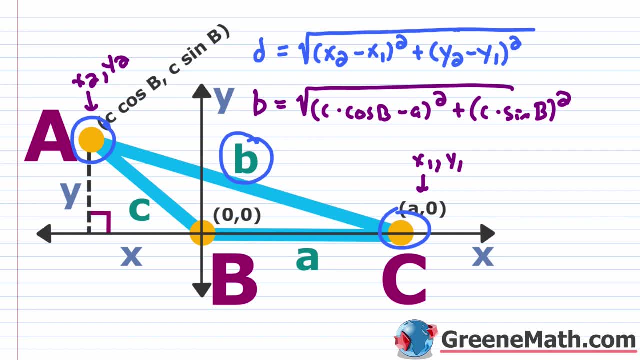 Let's go back up. I have things in terms of B squared right. So if I knew my side A and my side C and my angle here B- okay, my included angle- well then I could find the length of this guy B. 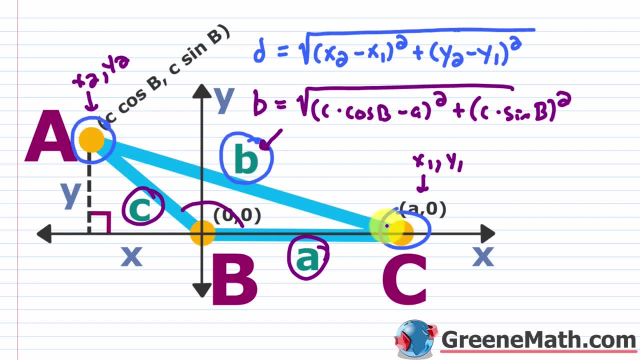 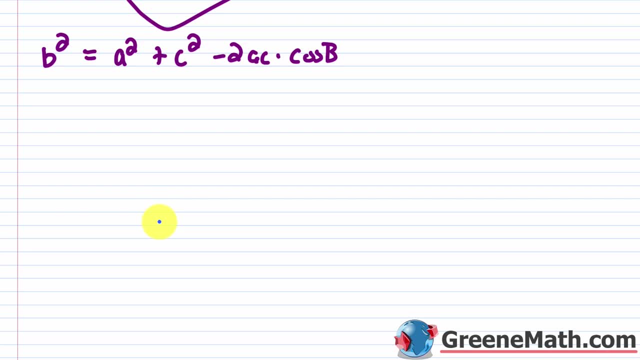 here, or the distance between these two points using that formula. okay, Now, additionally, we have two other forms and I'm not going to derive this. Obviously it would take forever, but you can do a similar process, So I'm going to do: A squared is equal to, in this particular case, 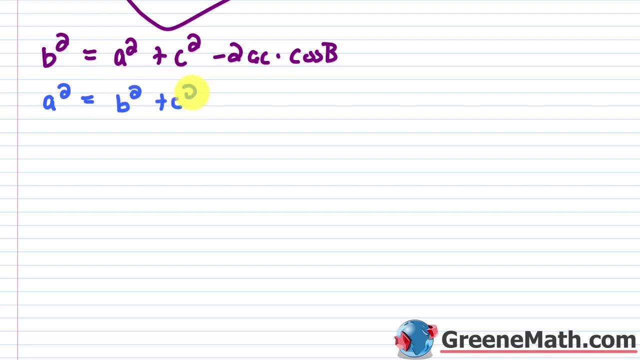 you're going to have B and C now, So B squared plus C squared and then minus. you'll have two times B times C, times the cosine of A. okay, And I think you see the pattern right. So basically you think about the side. 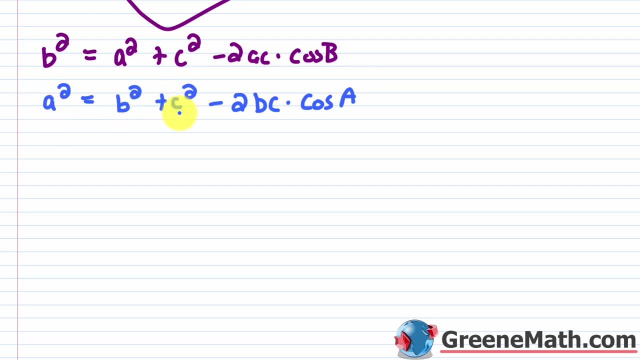 that you are solving, for It's the other two sides that you're going to need right. So B and C in this case, and you get B and C here, and it's the cosine of the angle A, opposite of this side, A. 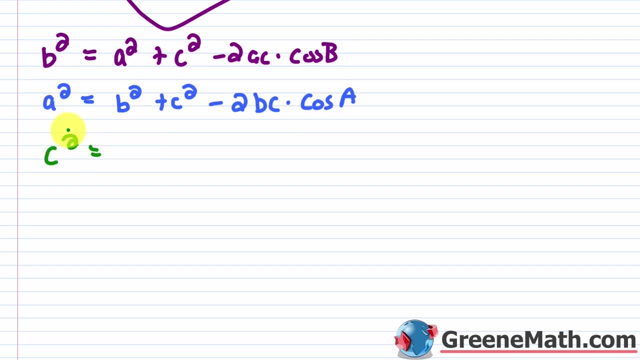 And then the last one. you probably guessed it. So C squared is equal to. you're going to have A and B now. So A squared plus B squared, minus, two times A, B Times, the cosine of, again opposite of C would be big C, cosine of capital letter C. 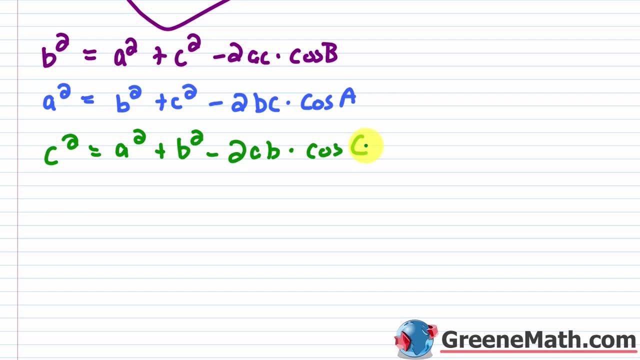 however, you want to think about that. So to give a little summary of this little law of cosines, we're going to say that the square of a side of a triangle is equal to the sum of the squares of the other two sides. Then you could go less twice the product of the two sides and the cosine of. 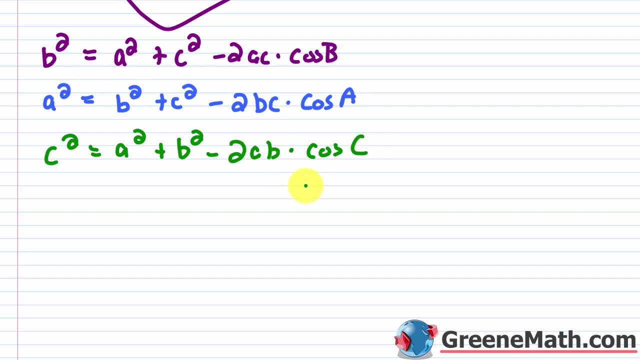 the included angle. okay, So this is a very easy pattern to memorize. Just go ahead and write it down in your notes. We're going to use it today. Okay, let's look at some examples. So let's go ahead and write it down in your notes. We're going to use it today. Okay, let's look at some. 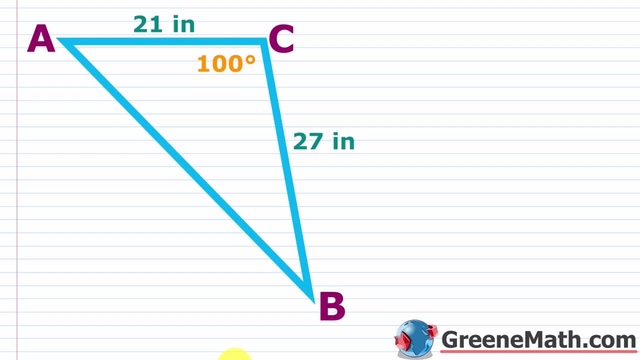 examples here. I'm going to do two with side angle side and then two with the side side side And then we'll look at some Heron's formula area problems. So the first thing you'll notice here is you have side angle, side right. So I have side B is 21 inches. I have angle C is 100. 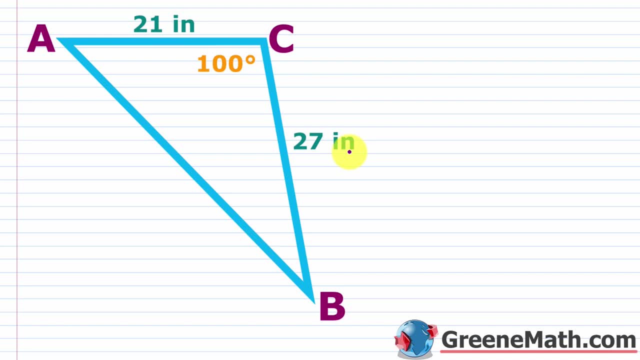 degrees and I have side A is 27 inches, So let's go ahead and write this down. So we had B was equal to 21 inches, okay. We had A was equal to it was 27 inches, Okay. so we have B was equal to, it was 27 inches And then we have side A was equal to it was. 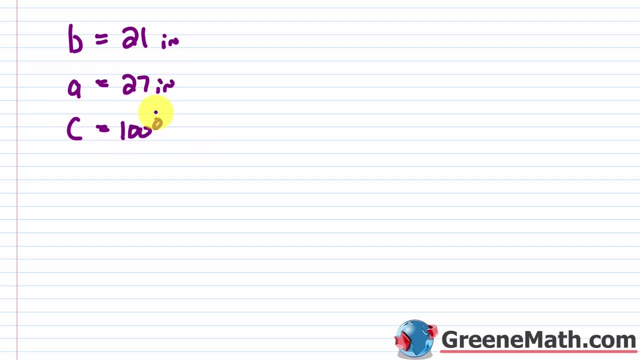 And then we had angle C was 100 degrees. okay, So with this guy, again, what you're trying to do in this particular case, you're trying to figure out when you start what is the missing side, right? So what is this C over here? What is this? So equals what? So let's come back, Okay. 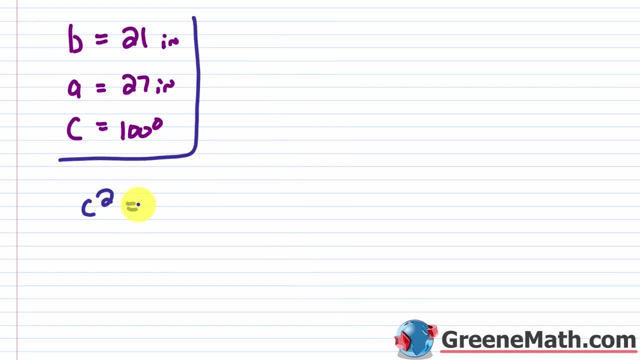 we're just going to plug into it. It's very simple. So C squared is equal to- hopefully you didn't forget this- So it's the two other guys. So it'd be A squared plus B squared. okay, Then minus it's two times this guy times this guy, So two times A. 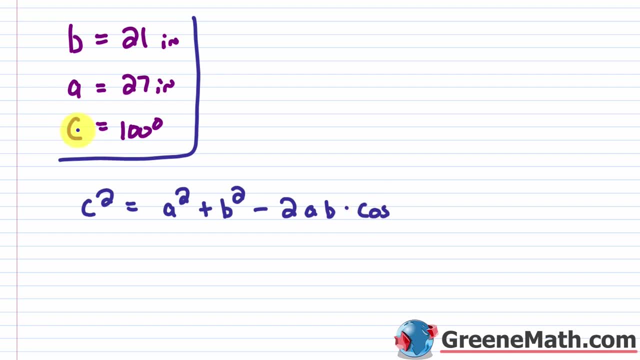 times B and then times the cosine of this angle here that you have, So the cosine of C. okay, Once you work with this a few times, it becomes very, very easy to remember it And you're just going to plug in and basically hit this on a calculator and you're done. 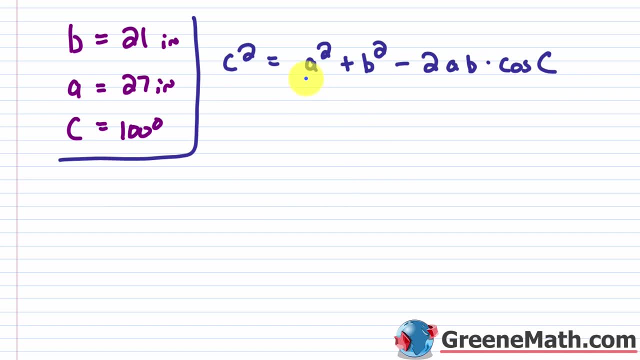 okay, So let me show you what you're going to plug in here and we'll approximate it together. You know that you want C by itself, okay, And C is going to be positive, right? So we don't need to consider plus or minus square root, So I'm just going to say C is equal to. 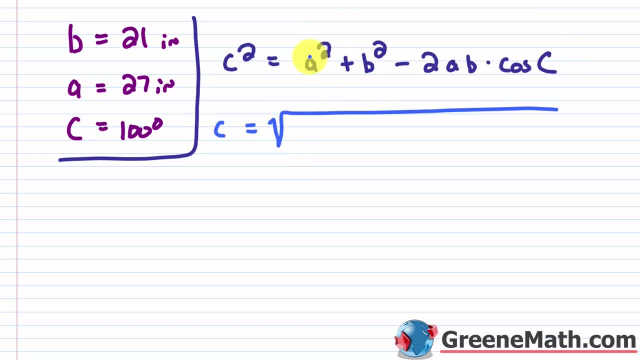 the square root of all of this. okay, So let me grab that. And I meant to just grab this part and it doesn't seem to be doing that, So let me write it: A squared plus B, squared minus two AB, and then times the cosine of C. okay, So C is equal to the square root of. 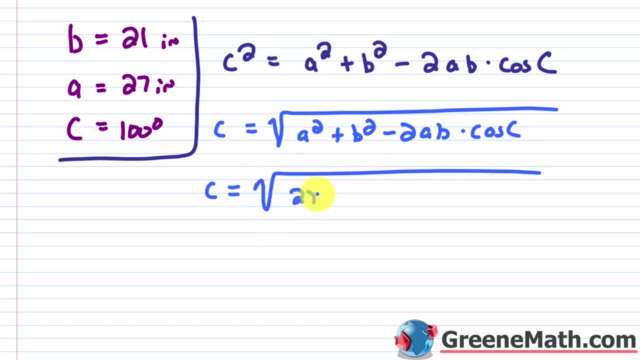 let's plug in here. So for A, I'm going to plug in 27,. okay, You can put the units in if you want or not. In the end it's going to come out to just be inches, So I'm just going to leave them off. 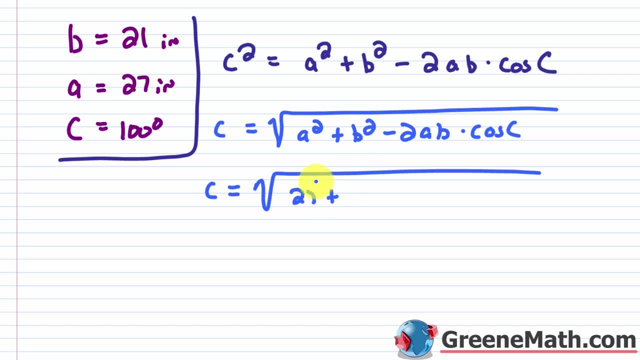 okay, Then plus for your B, it's going to be- and I forgot to square this- For your B, it's going to be 21.. So, 21 squared and then minus two times your 27.. Times your 21 and then times your cosine of 100, okay, Degrees. Now you're just going to punch. 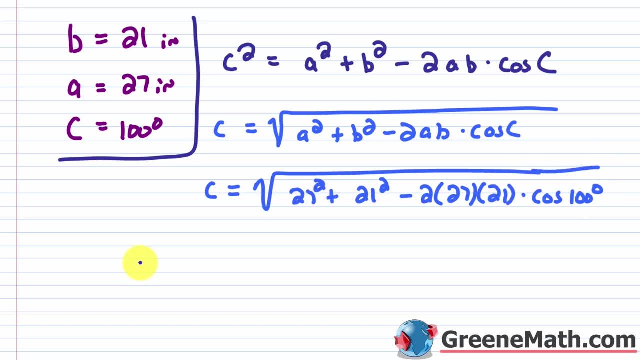 this into a calculator and I get about 36.97 and I'm going to do 37, okay, So I'm going to say my side C- okay, This is a lowercase, C is equal to 37, and then the units are inches. okay, All right. 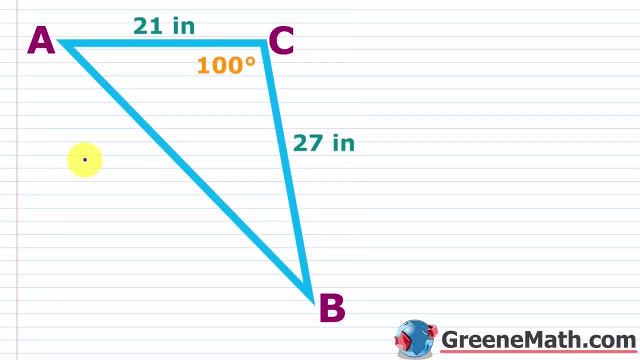 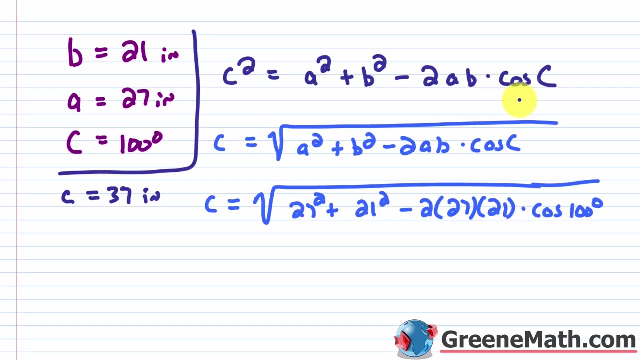 so let's erase this and let's put here that C is approximately 37 inches. Now let's define our two missing angles here, okay, And let's talk for a minute about using the law of sines or using the law of cosines. If you go back and you think about it, you can always 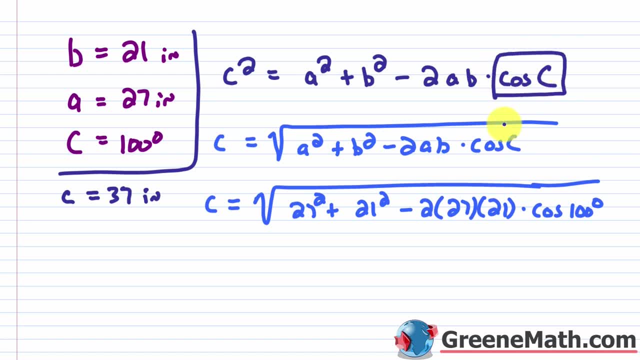 in any of these formulas, you can solve for this guy, okay, And you can end up using your inverse cosine function to solve, okay, So that's fine. If you want to use the law of sines, you have to be very, very careful. Why, Remember, if you have an obtuse angle and a triangle, you can only have 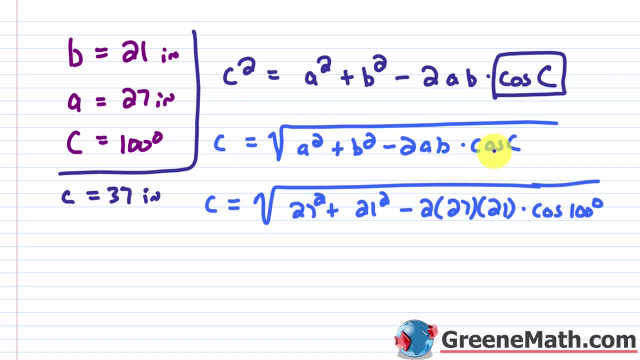 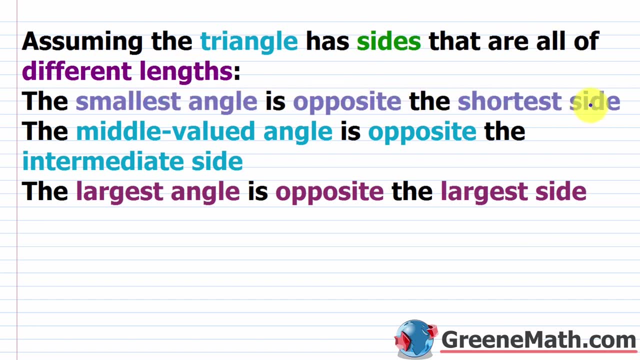 one of them okay, And it's going to be opposite, So you're going to have to use the law of sines. the largest side. If we go back here, remember, assuming the triangle has sides that are all of different lengths, the smallest angle is opposite the shortest side. the middle valued angle is 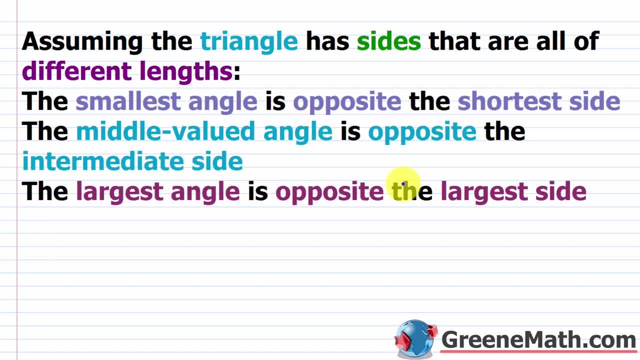 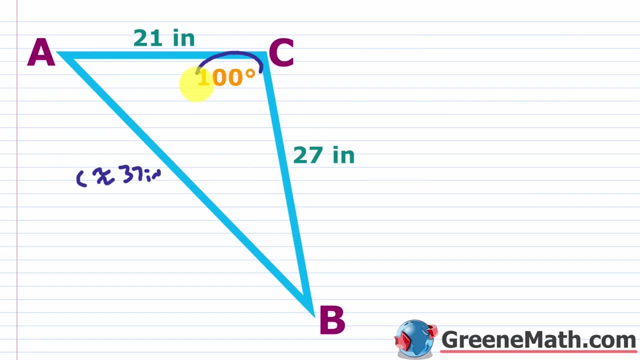 opposite the intermediate side and the largest angle is opposite the largest side. okay, So what am I getting at here? Well, basically, what's going to happen is, in this particular case, you have an obtuse angle already. okay, So it is opposite of the largest side, and we can clearly 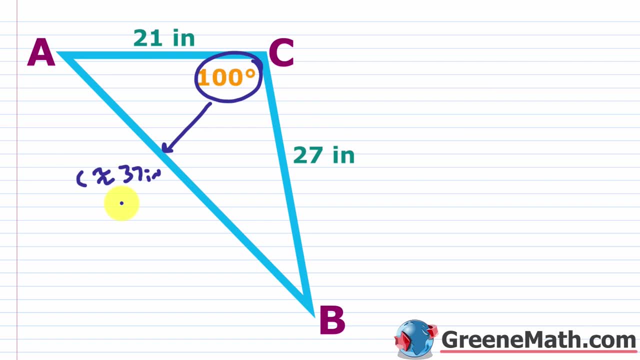 see that. But let's say that you didn't have an obtuse angle. Let's say you had an angle. that was well. when you go to find your other missing angles, if you're using the law of sines, you might run into a problem. okay, Because when you think about the inverse sine function, you can't get an. 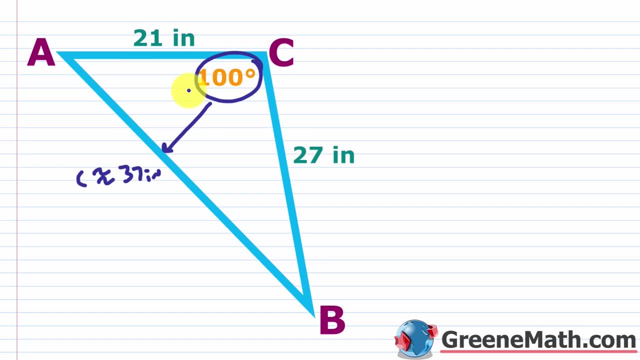 obtuse angle out of that. okay, You can't. You can only get something in terms of from quadrant one between zero and 90 degrees. okay, That's all you can do. So if you had something larger than 90 degrees, you would get the wrong answer right. So, for example, if the angle measure should be: 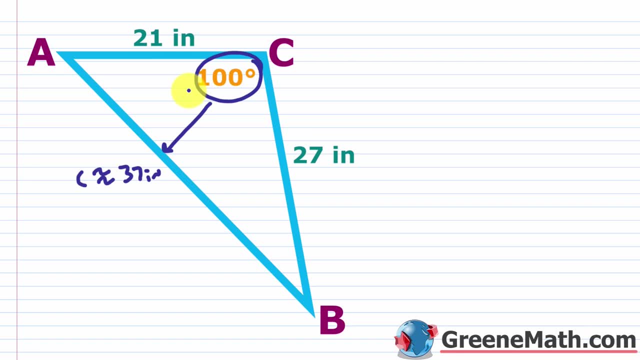 110 degrees. if you plug in the inverse sine function there, you would end up with 70 degrees. Okay, that's just how it works. So what we do to fix this is: we find the smaller of the two remaining angles using the law of sines. okay, Because if I find the smaller one, then it's not. 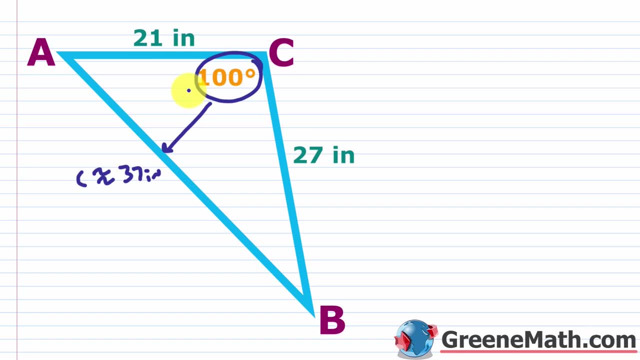 possible for it to be the obtuse angle, Because, again, a triangle can only have one obtuse angle. So if I'm finding the smaller one, it can't be that one. So I'm good to go to use the law of sines, okay, So let's go ahead and find the angle measure B right, Because it's opposite the 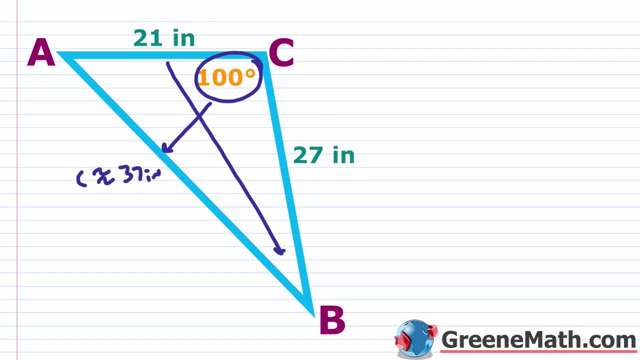 smaller side right. This one's 21,, this one's 27,. okay, So let's go ahead and find the angle measure B, Let's go back and let's go ahead and say that we have the sine of, in this case, C, which is 100. 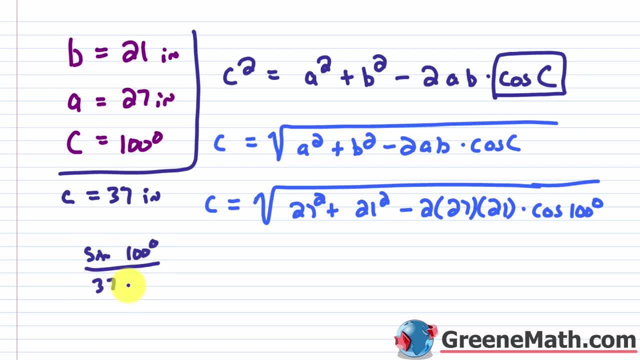 degrees, okay. over C, which is 37 inches, is equal to: the sine of B over B is 21 inches, okay, So we already know how this is going to work. We're basically going to multiply both sides by 21 inches, So we'll say that the sine of B, the sine of B, is equal to. we'll have 21 inches. 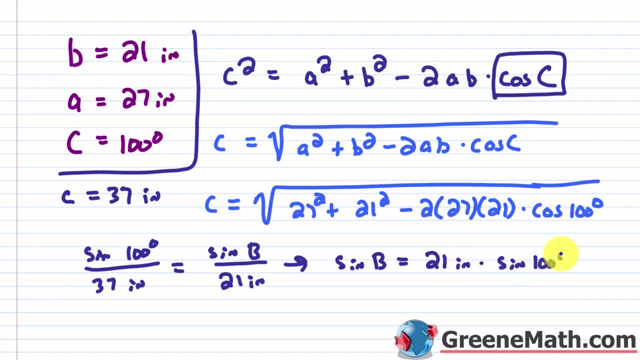 times, you're going to have the sine of 100 degrees, So we're going to multiply both sides degrees. This is all over your 37 inches, okay, And you can go ahead and cancel the units inches out if you want. visibly, Just punch this into your calculator and you're going to find that the sine 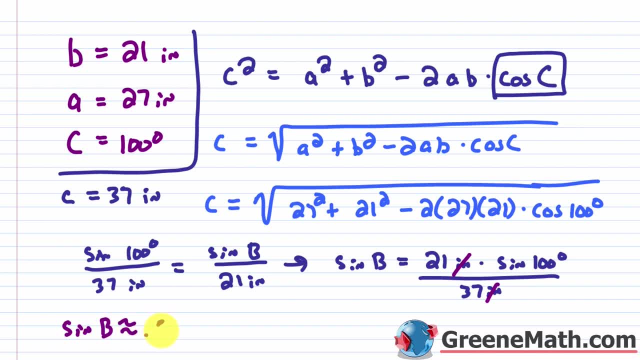 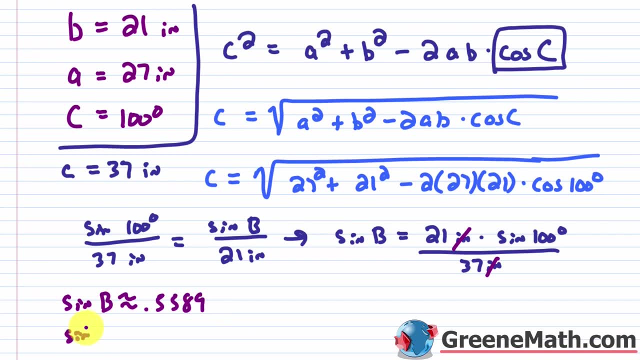 of B is approximately, let's just say it's 0.55,. I'll just say 89,. okay, So if you use your inverse sine function on this, I'll say sine inverse of this, 0.5589,. this is approximately. we'll say: 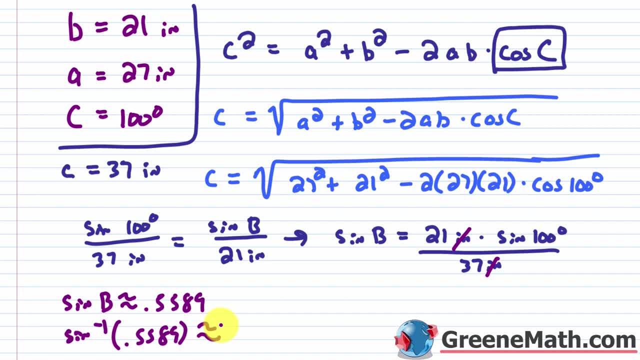 33.98.. So I'm going to say 0.5589.. So I'm going to say 0.5589.. So I'm going to say 0.5589.. So I'm all around at the 34.. So I'll say this is about 34 degrees. okay, So that would be your measure. 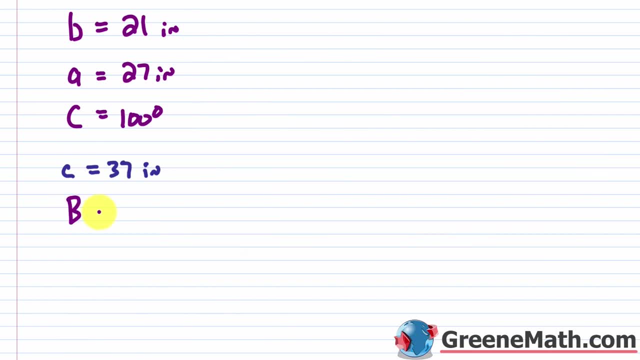 for angle B. So let's erase all this and I'll say that B is approximately 34 degrees, And then to find A, all you have to do is subtract, right, So you're going to do 180 degrees, basically minus your 100 degrees. okay, So that would be 80 degrees and then minus your 34 degrees, which. 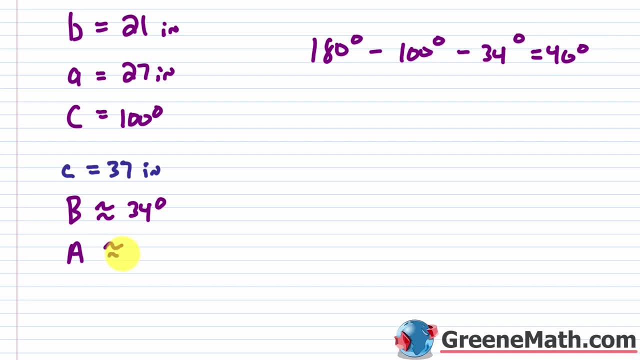 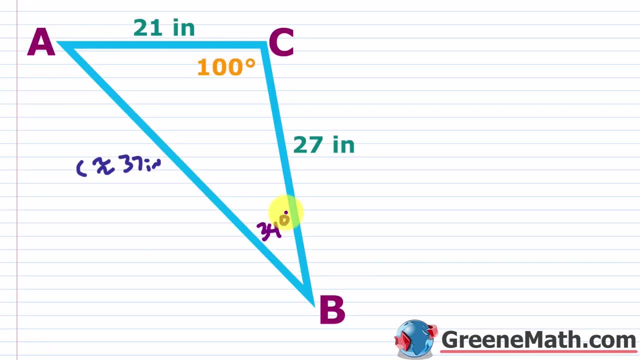 would give me 46 degrees. okay, So A is approximately 46 degrees. okay, So we've solved this guy. Let's go back up and I'll just say this is 34 degrees and I'll say this is 46 degrees. All right, let's look at another example with side angle side. I'll go faster on this one. 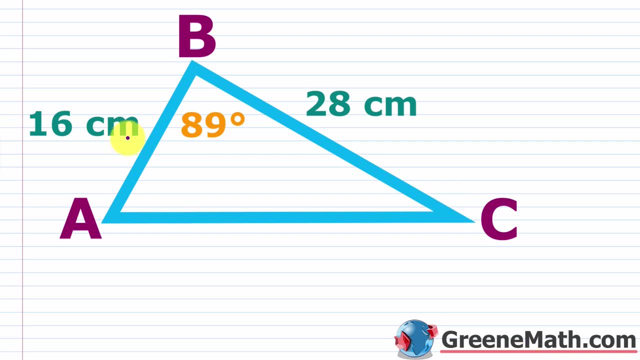 So basically here you have a side C that's 16 centimeters, You have an angle B that's 89 degrees and you have a side A that's 28 centimeters. So let's say C is 16 centimeters, Let's say that angle B- sorry I was writing A, but angle B is 89 degrees. 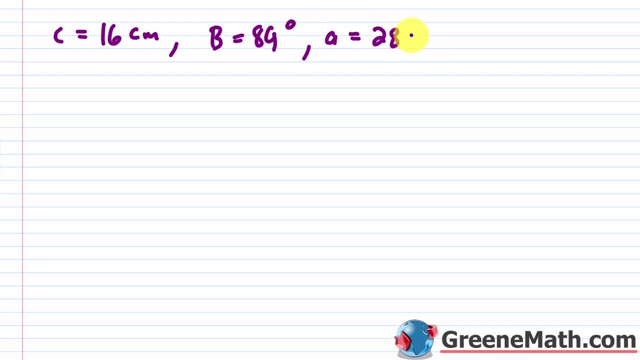 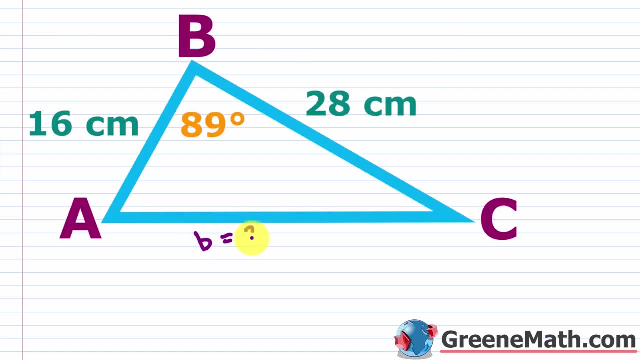 And then let's say that side A is going to be 28 centimeters. okay, So again, the first thing I want to do is find the missing side right. So we're going to say B is equal to Y, So again, 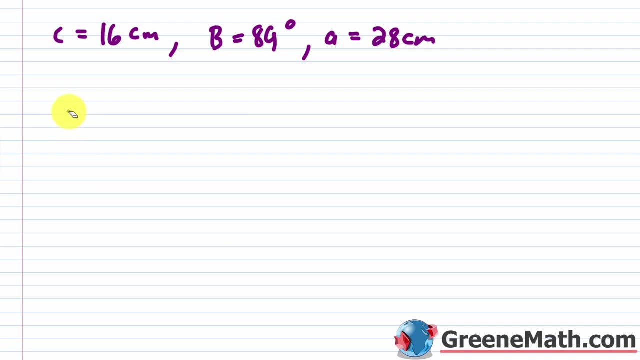 just use your law of cosines, very easy. So we're going to say B squared, So B squared is equal to again, which ones are not involved. So it's going to be A and C, So A squared plus C squared, and 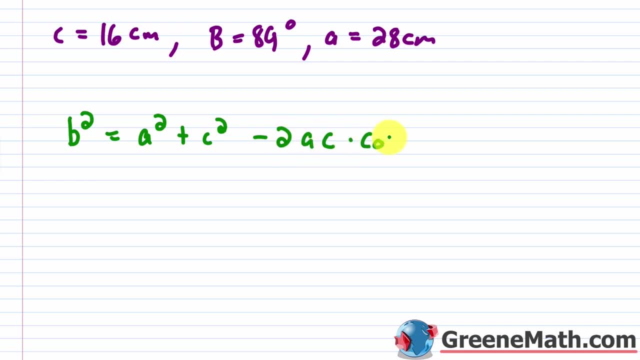 then minus two times A, times C, times the cosine of this angle here, which is B. okay, So we're just going to plug in. So let's just go ahead and say: this is B is equal to the square root of. I'm going to plug in for A, that's going to be 28.. And forget about the units you don't really need. 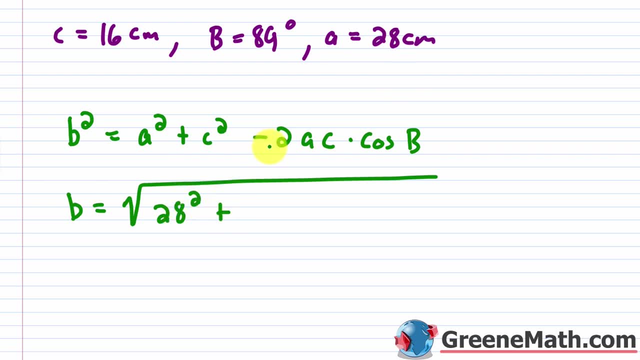 them, because it's going to end up just being centimeters. So then, plus for the C, it's going to be 16. And then for the minus, two times again it's going to be, and this needs to be squared. 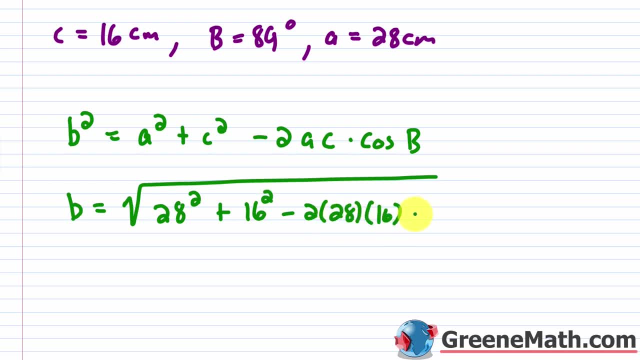 two times, for this is going to be 28, and then times 16 and then times the cosine of- in this case it's 89 degrees. okay, So I'm going to go into a calculator So I get about 32, let's just call it that. So I'll say: 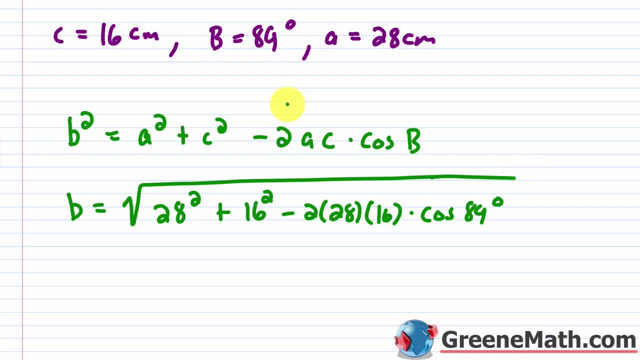 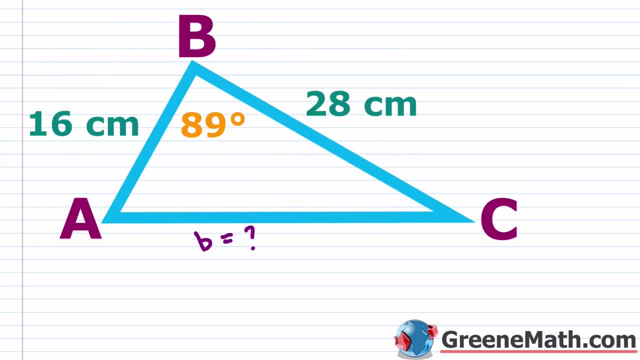 it's about 32 centimeters. So we'll come here and we'll say that our side B is approximately 32 centimeters. And again, if we go back up here we can just label this. I'll say: this is approximately 32 centimeters. And again, you just want to take out of these two sides here, you want to take the. 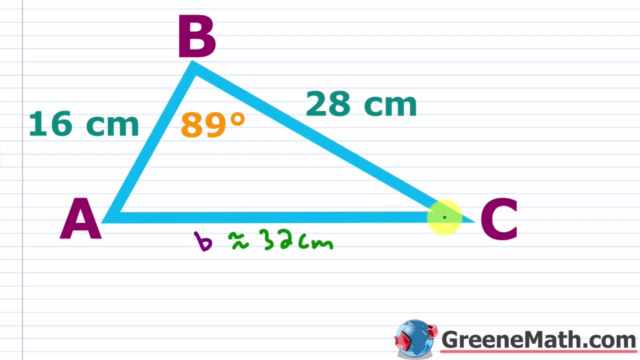 smaller side, okay, And then go opposite. you want to find that angle measure. So I'm looking for angle C here because, again, if I go back up here I'm going to find that angle measure. So I'm not going to be obtuse. it's not possible. So I can use my law of sines. If you want to use the. 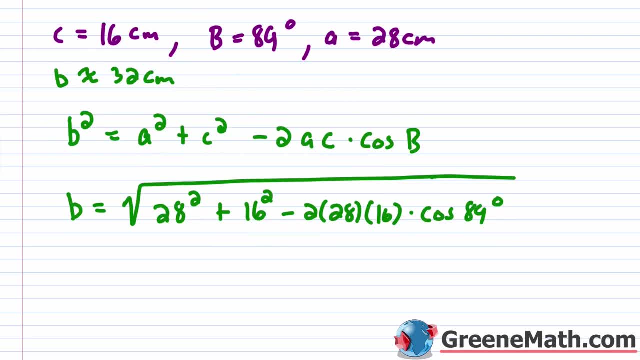 law of cosines. you can do that as well. It's up to you, okay. So let's go back and let's figure out angle C. So I'm just going to say the sine of C is equal to. so I'm going to write 16 centimeters. 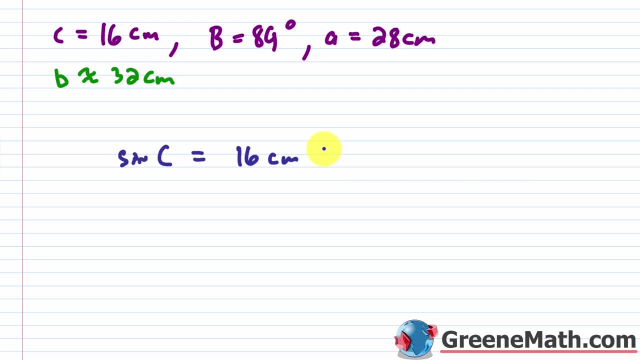 here And again you can leave the units off because you know you're going to end up canceling them out, but I'll just show it here. And then times it's going to be basically the sine of 89 degrees, which is basically B. okay, Over B, which is: 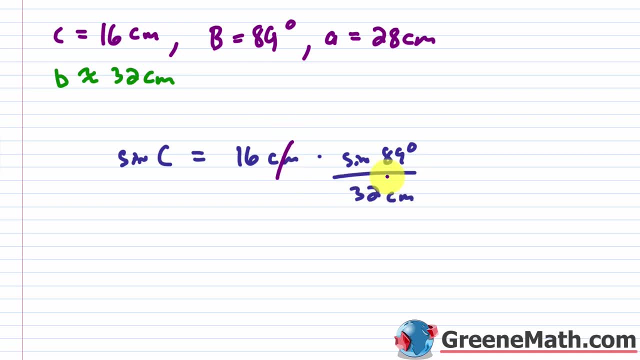 in this case 32 centimeters. okay, I'm going to visibly cancel these units. punch this into a calculator and you'll see that the sine of C is approximately, I would say, 0.4999,. let's just call. 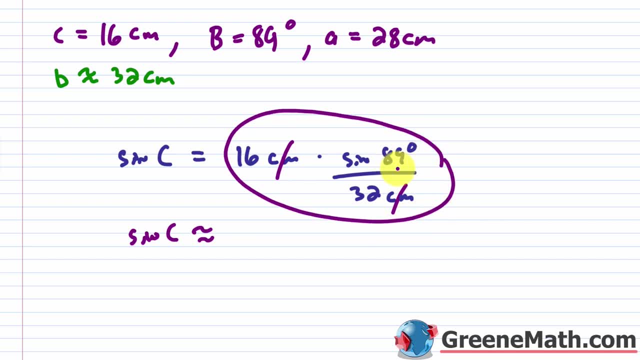 it that? But if you wanted to make this a little quicker, you just take this whole thing, plug it into your calculator for the inverse sine function and you'll have C. okay, I'm just doing this in two steps to make it a little bit easier to comprehend. So 0.4999, and then I'll say sine. 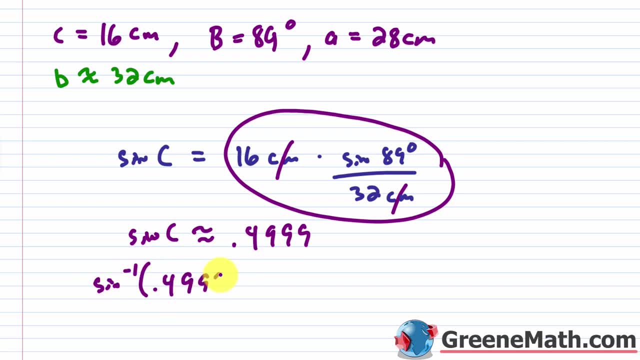 inverse of this guy: 0.4999.. 0.4999 would be approximately. let's say it's about 30 degrees okay. So that would be for C, okay. So let's erase this. So we'll say C is about 30 degrees, okay, And then again, if you want to, 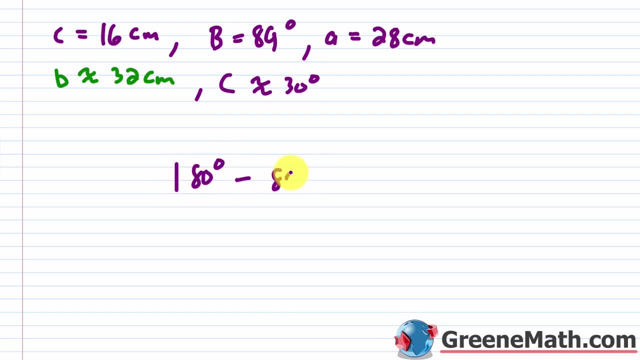 find A, you're going to do 180 degrees minus 89 degrees minus 30 degrees, which is 61 degrees. So I'll say that A is approximately okay. I'll say 61 degrees, So we'll say this is about 61. 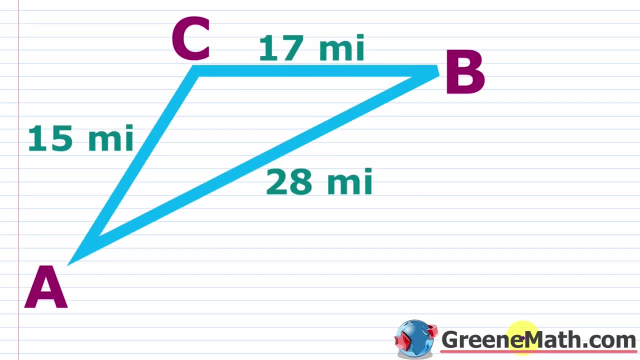 degrees and we'll say this one is about 30 degrees. All right, let's change things up just a little bit and look at the case where we have the side, side, side, So we have all three sides and to solve the triangle you need to find the three. 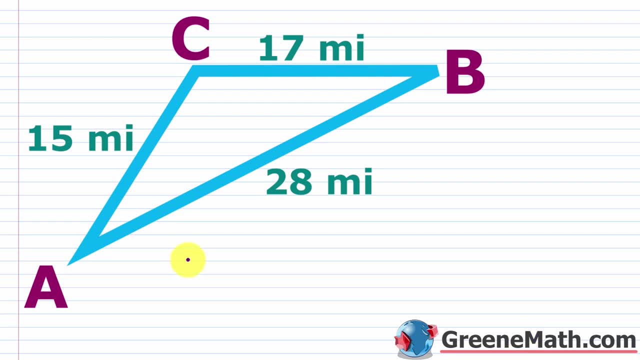 missing angles. So in this particular case, let me just read this off: We have our side A, which is going to be 17 miles- Let me make this equal sign a little bit better, okay. And then we have our side B- our side B, which is going to be 15 miles. And then we have our side C. 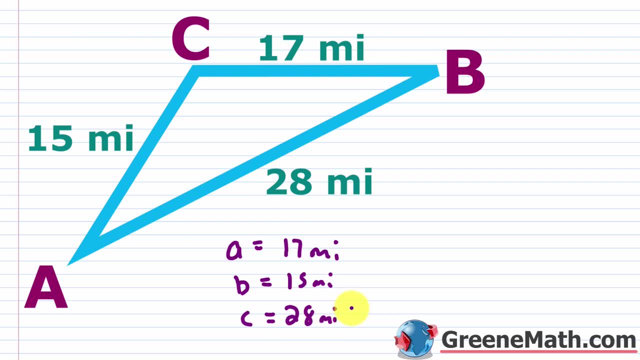 lastly, which is going to be 28. miles. okay, So, based on the information about a triangle that we know, we know that this angle C here would be the largest angle. okay, Because it's opposite of this largest side. okay, So when? 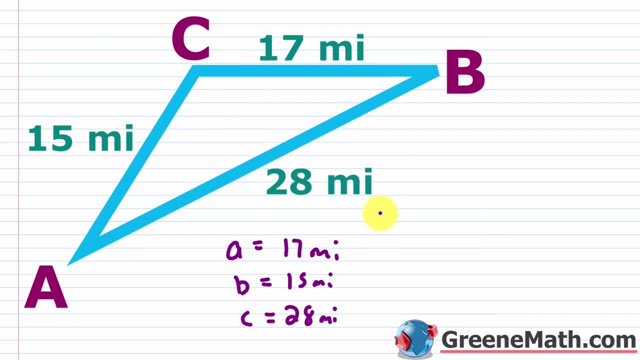 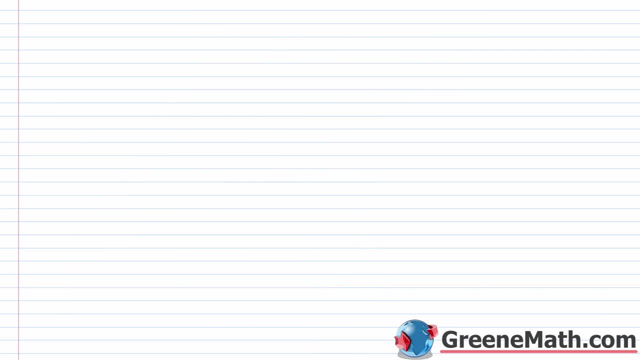 you have all three sides. you're going to first find the largest angle using your law of cosines, okay, So let me grab this real quick. Let me cut it away. Let's come to a fresh sheet, so we have a lot of room to work, okay, And I'm going to be focusing on finding our C. So what is this guy? 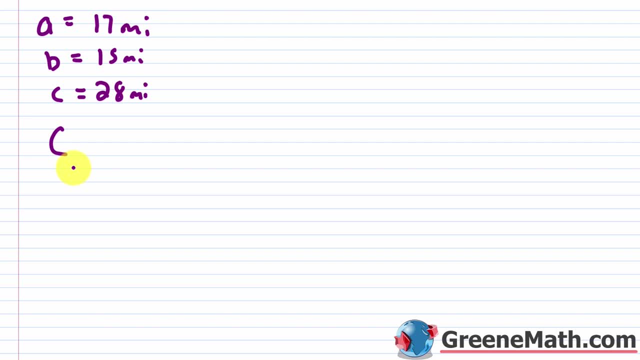 What is the measure? So let's turn back to our law of cosines, and I'm going to use the one with the cosine of C involved. So, in other words, let me just erase this real quick. so I have some room, Let me box. 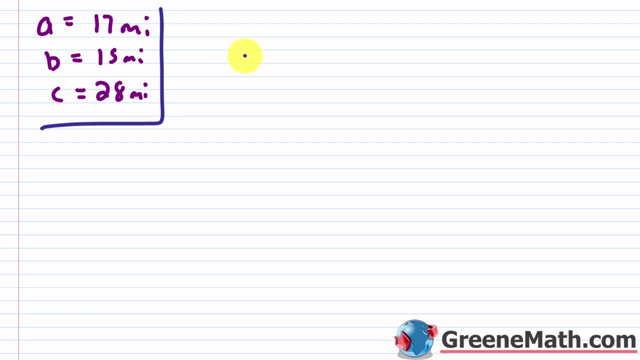 this off. I'm going to say- or actually I can actually do this up here- I'm going to say that C squared is equal. to remember. take the other ones that aren't involved. So you're going to have A squared plus your B squared and minus 2 times A times B, okay, times the cosine of C. 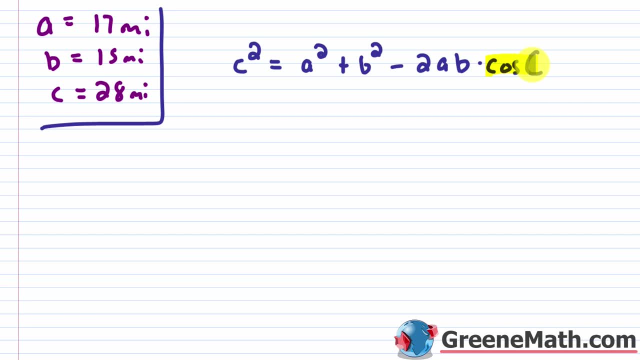 So the idea here is that you're going to isolate the cosine of C- okay, So it's going to be equal to something. okay, You're going to be able to plug in for A, B and C here, okay, And so then you can use your inverse cosine function and find out what C is. 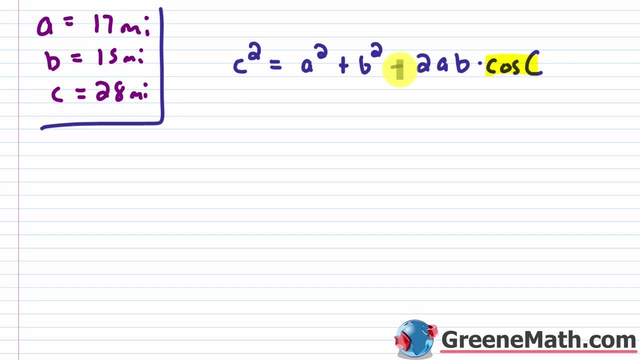 approximately Now, when you talk about the law of sines, again with the inverse sine function, you run into problems because the inverse sine function is not going to be able to give you something in quadrant two right, So you're not going to be able to get an obtuse angle out of. 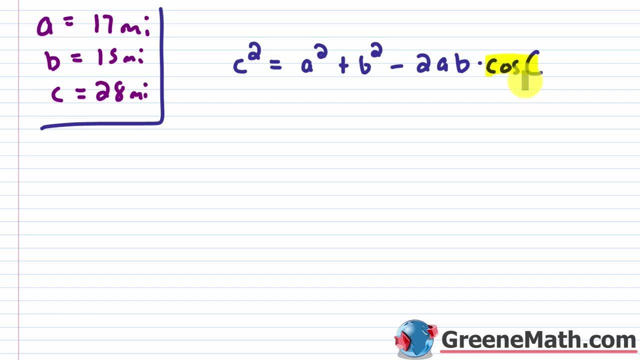 that With the inverse cosine function you can right. It returns something from zero to pi in radians or from zero to 180 degrees. So if you get a negative cosine value, you know you're in quadrant two and you have an obtuse angle. If you get a positive cosine value, okay, you're in. 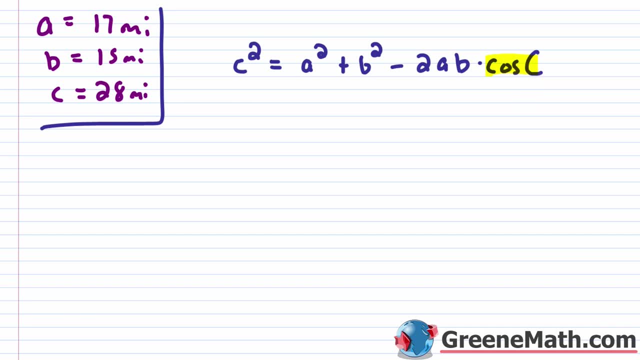 quadrant one, and so you have an acute angle. okay, Let's quickly solve this guy. for the cosine of C In the next example, I'll just give you the formula, but I just want you to see where this comes from in your book. So the first thing I would do is I would subtract A squared and I: 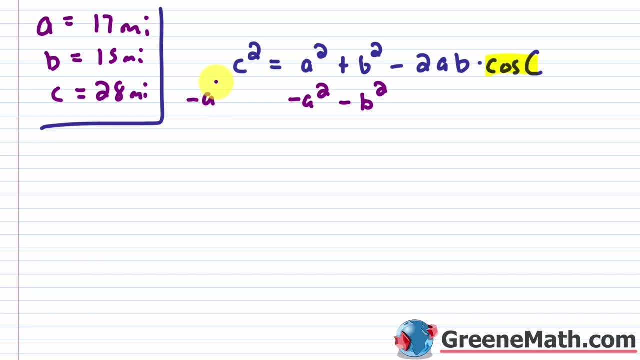 would subtract B squared away from each side. okay, So minus A squared and then minus B squared. So it's going to cancel over here. Let me write this down here. I'll say: we have C squared minus A squared. minus B squared is equal to the negative of 2AB times the cosine of C. okay, This is. 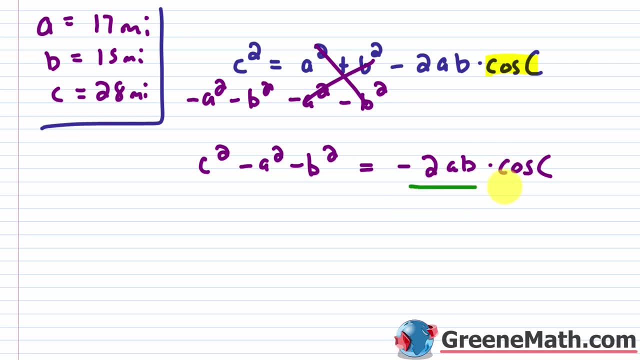 multiplication here. So what I'm going to do to isolate this, I'm going to divide both sides by negative 2AB. okay, So divide both sides by negative 2AB. Let me erase this from up here so we can write this formula up here. This is, of course, going to cancel, So that's gone. 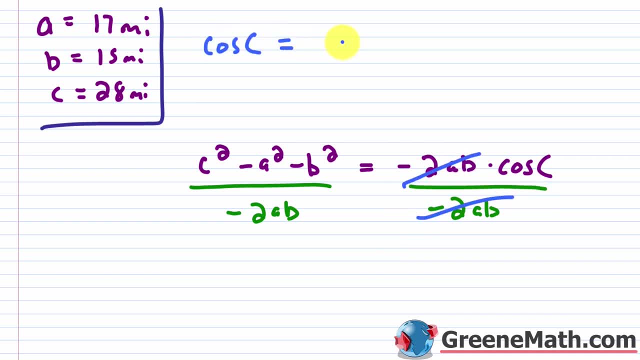 So you'll have the cosine of C is equal to. you'll have your C squared over here, C squared minus A, squared minus B, squared over the negative of 2AB. Now, because this is a fraction, I can keep my negative down here, or I can get rid of it and I can bring it up to the top. 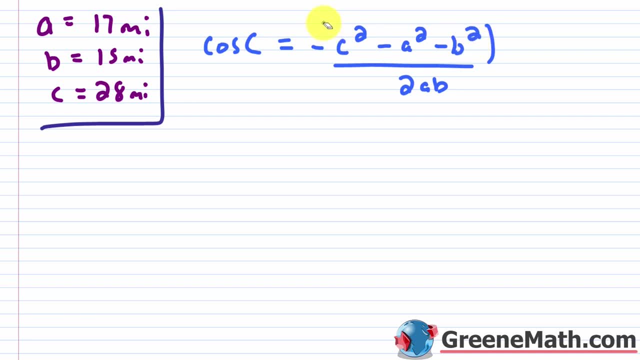 like this right, So I could distribute it to each part, So I could say: this is negative C squared plus A squared plus B squared. okay, like this. And then I'm going to rearrange it, So I'm going to say: and this is how it's going to be in your book, so that's why I'm doing this. So the cosine. 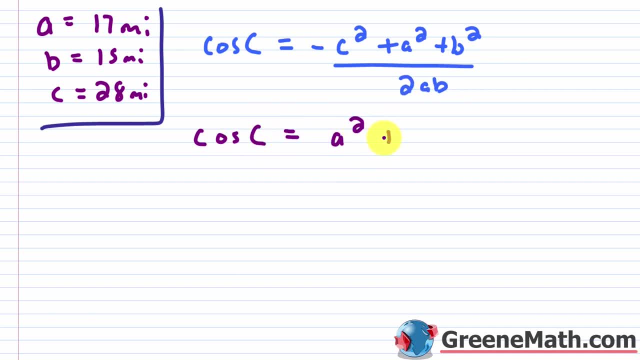 of C is equal to, I'll say: this is A squared plus B squared. okay, like this. And then I'm going to. I know it takes a while to get these things And in tutorials we're used to just being given the. 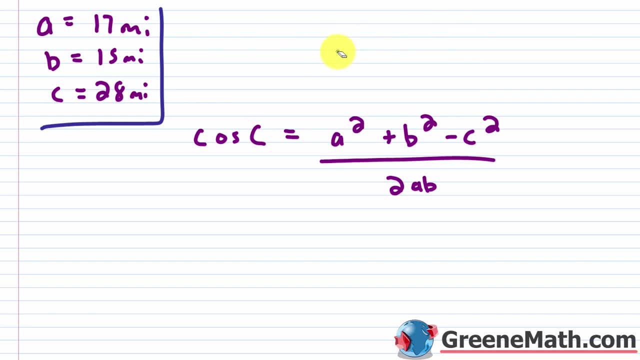 formula, But I want you to see where things are coming from in your book, So you're not always just getting things handy, Okay, so let me grab this up here And basically now I'm just going to plug in, okay, And to make this quicker. if you wanted to, you could just do the inverse cosine. 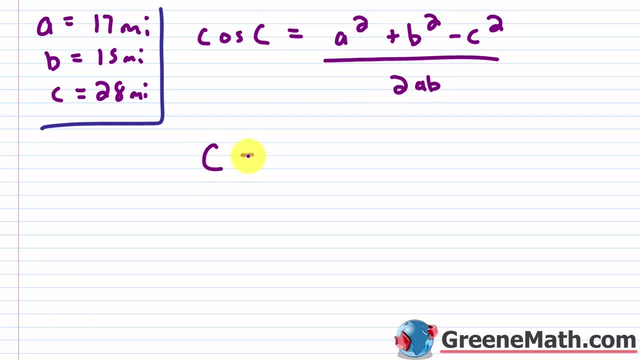 of whatever this is. to give you C right. So you could say: C is equal to the cosine inverse of. so I'm just going to plug in here. So I'm going to plug in here. So I'm going to plug in here. 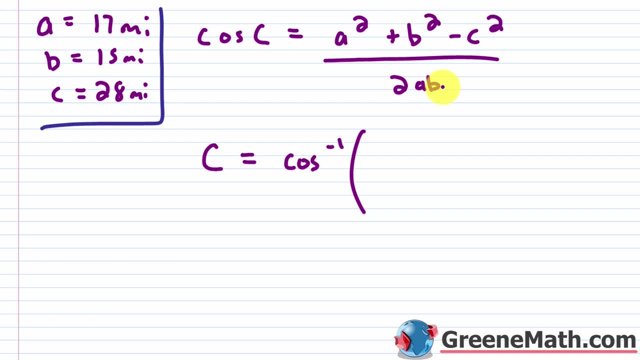 I'm just going to plug in for A, B and C here. You can leave your units off. you know they're going to cancel. So A is going to be 17.. So that's squared. plus B is going to be 15, that's squared. 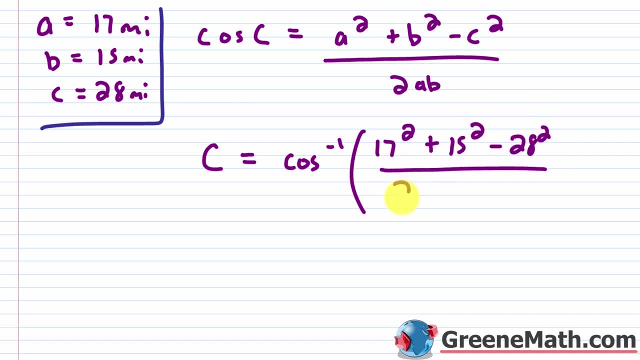 minus C is going to be 28,. that's squared all over two times. you're going to have your 17, and then times your 15.. Okay, so just punch this into a calculator, use your cosine inverse function And let's say that's about 122 degrees. okay, if we ran to the nearest 10.. So I'll say: 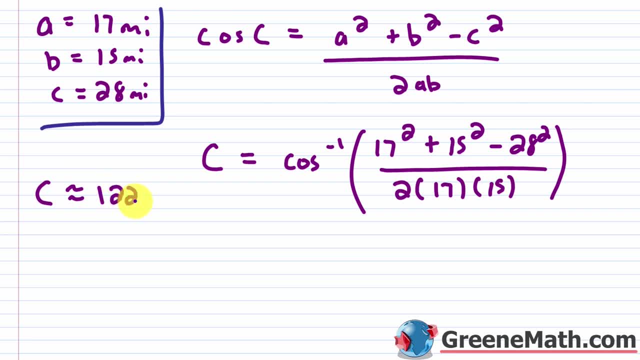 here that C is approximately 122 degrees. okay, And if you look at this value right here, you'll notice that this guy is negative. okay, So if the cosine value is negative, you're going to get an obtuse angle right. 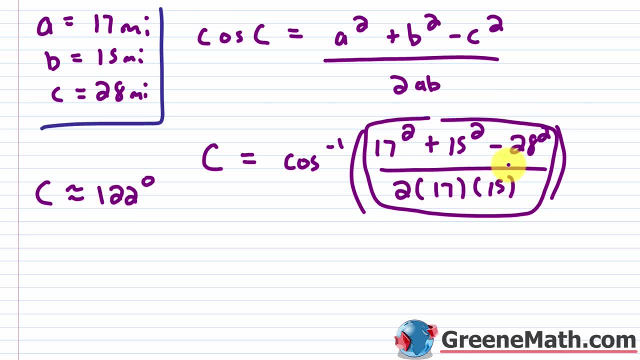 because you're getting something in quadrant two. If this guy ends up being positive, you're going to be in quadrant one and you're going to have an acute angle. okay, But you see how you avoid that problem, versus when you're working with the law of sines. right there you really have to be. 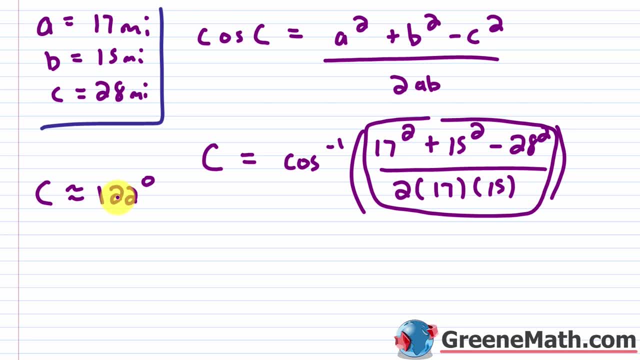 careful about what you're doing. So now that we have the largest angle, when I think about the angle A or the angle B, I'm going to have the largest angle and I'm going to have the largest angle B. they have to be acute angles, right? If you always find the first angle as the largest. 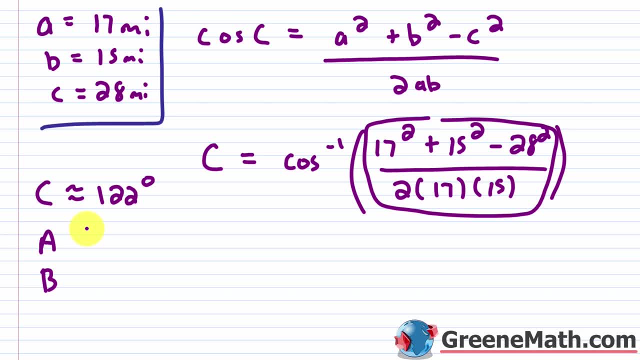 angle. then you don't have to worry about the next two angles, you can just use the law of sines, okay? So let me get rid of this And let's just use our law of sines here, real quick. So I'm going. 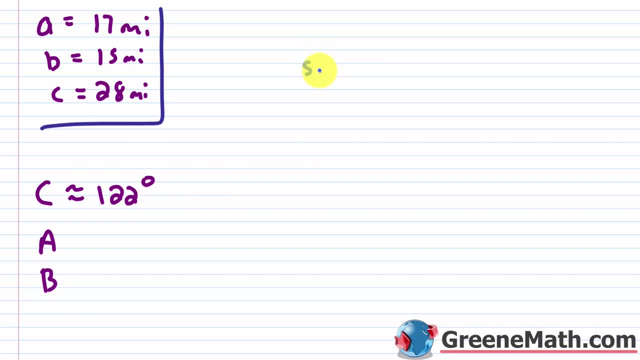 to say in each case that I have the sine of, in this case, 122 degrees over whatever C is, which is 28 miles. again, you can write the units if you want. it's going to end up canceling, So 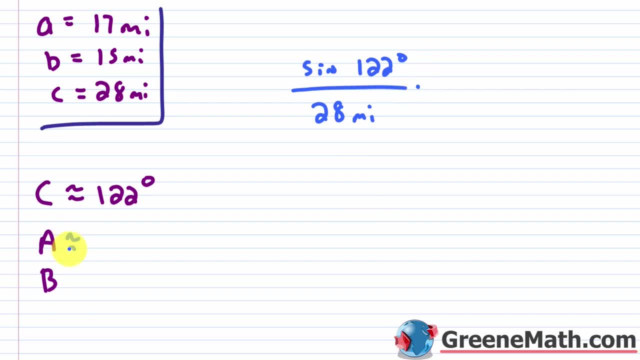 I'm going to multiply this by 122 degrees and I'm going to have the sine of 122 degrees and I'm going to multiply it. let's just start with A. we'll say it's approximately what. So let me go. 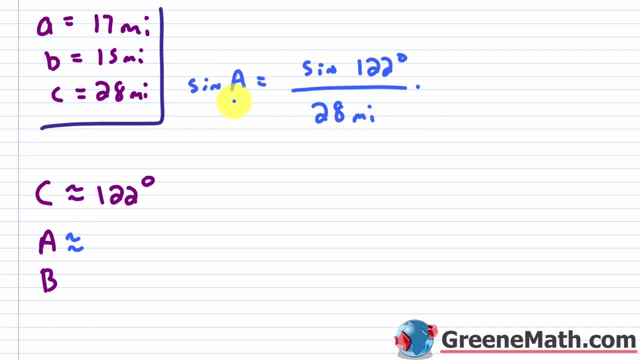 the sine of A is equal to this. So I'm going to multiply this by what I would have divided by here, which is 17 miles. okay, So you can see that this is going to cancel here. then, to make this a little bit quicker, let's just go ahead and say A is going to be equal to. we're going to do our. 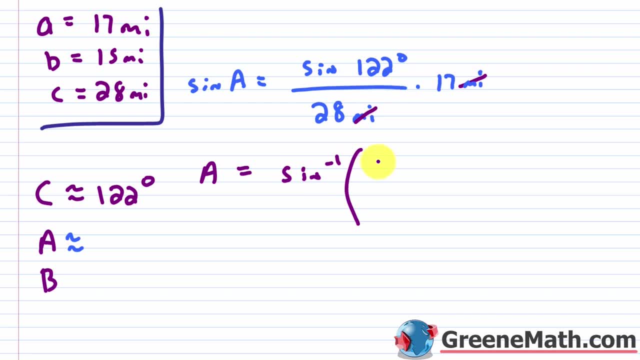 inverse, sine function, So sine inverse of this whole thing. So the sine of 122 degrees over 28,, then times 17,. okay, like this. So if we punch that into a calculator you're going to get a about 31 degrees. So let's say A is about 31 degrees, okay. And then, once you have those two, 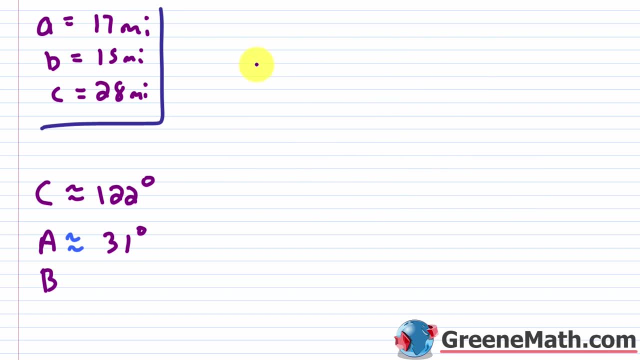 again you could just use the angle sum property of a triangle. So again, 180 degrees is the sum of all the angles and make that zero a little bit better. Then minus you've got this one is 122 degrees. then minus you got this one is 31 degrees. you can just say this is 27 degrees. 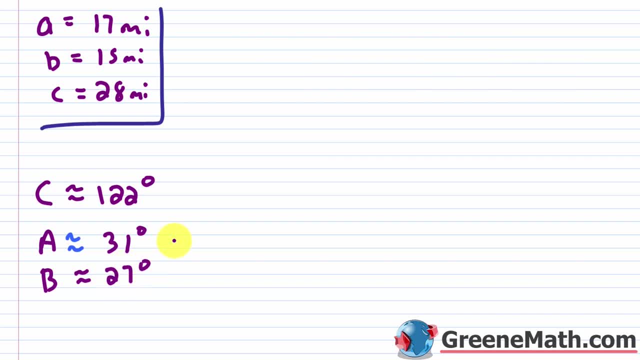 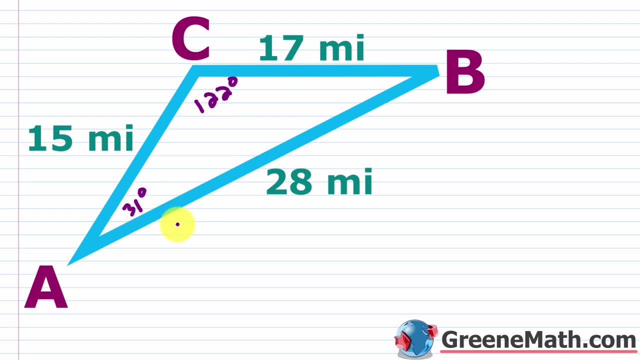 okay, So this is about 27 degrees. So let's go back up And I'll say: C is 122 degrees. Again, this is an approximation: A is about 31 degrees And B is about 27 degrees. Okay, let's look at one more example. I'll go a little bit quicker. 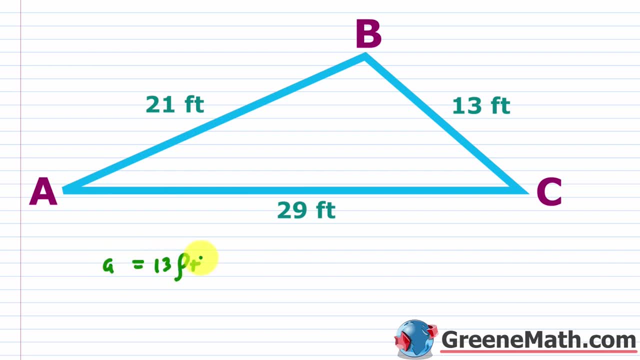 through this one. So we'll say A is 13 feet, okay, And then you could say B is going to be 29 feet, And then C is going to be 21 feet, Okay. so let me grab this And let's paste this in Again. 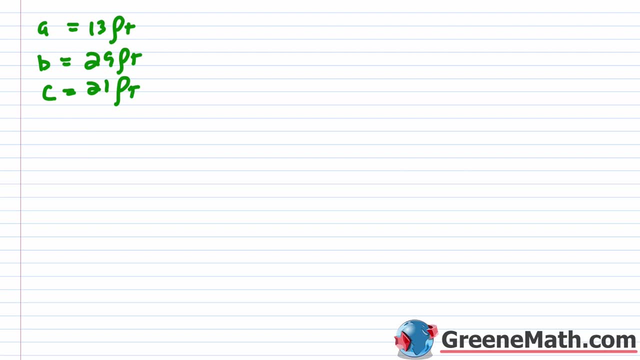 you're going to work with your largest angle first, So look for your largest size. That's going to be here, right? So we're gonna be looking for B. So I'm just going to give you this formula You wrote out: the B squared is equal to A squared plus C squared minus two times A times C, times the. 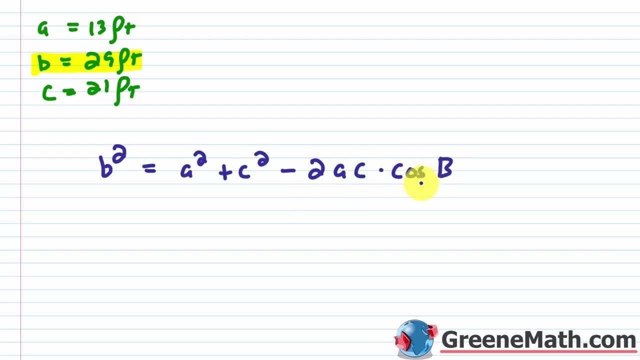 cosine of B. okay, And you solved it for the cosine of B you're going to end up with. the cosine of B is equal to, we'll say, A squared plus C squared minus B, squared all over your 2AC. Okay. so let's. 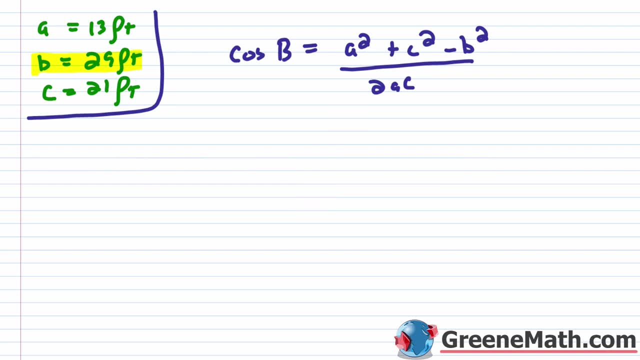 get rid of this. And again, if you really wanted to take this forward, you could say that B is equal to the cosine inverse of. you can just grab this right here. So A squared plus C squared minus B squared over 2AC. Okay, so you can just plug in like this and basically find out what B. 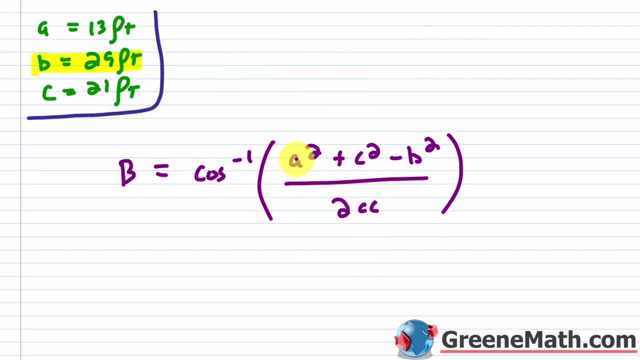 is approximately Alright, so let's plug in. For A, we have 13 feet, So we have. let me change colors here. We have 13 feet, I'm just gonna put 13,. forget about the units. So for C, I'm gonna put. 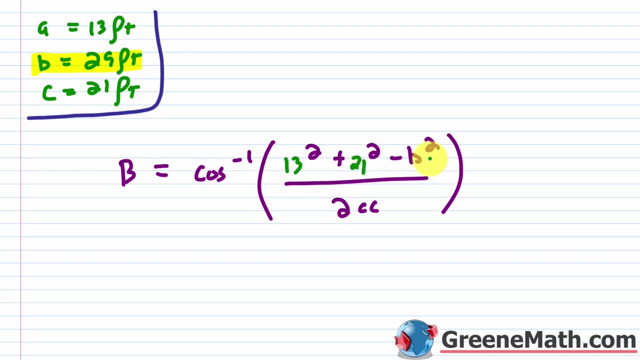 21.. So put 21.. And then for B, I'm gonna put 29.. So let's put 29 there. And then two times B, two times A times C, So A is 13. And C is going to be 21.. Okay, so let's punch this into the. 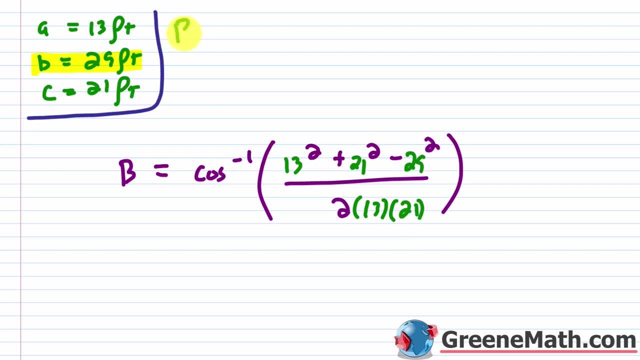 calculator And I get about 115 degrees. So B is approximately 115 degrees. Okay, let's erase this. And again, I've got my obtuse angle, Okay. so once I have my obtuse angle, the other ones are going. 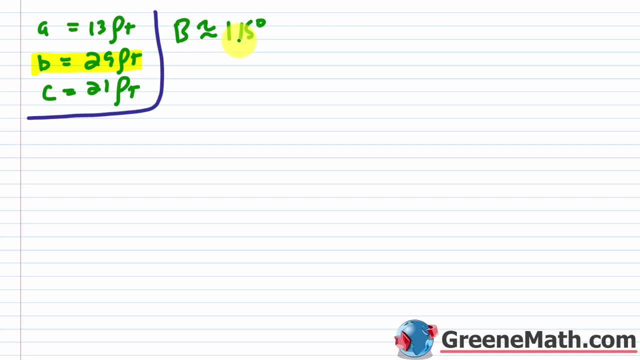 to be acute for sure. Okay, so I don't have to worry about the law of sines. right, It's not going to give me an error if I use that now. Alright, so let's solve for A. So we have the. 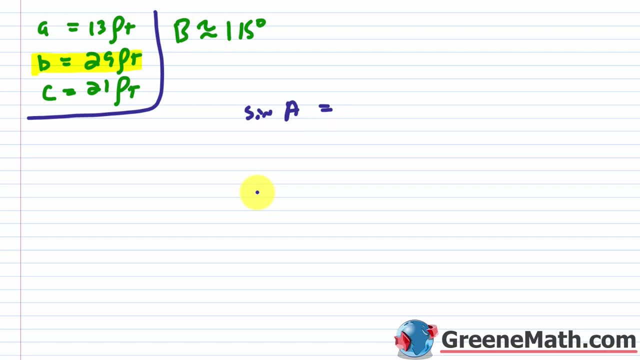 sine of A is equal to we go A, which is basically 13 feet times- let me make that three a little bit better times. we're going to go the sine of B, So the sine of 115 degrees, And this is all over B itself, which is 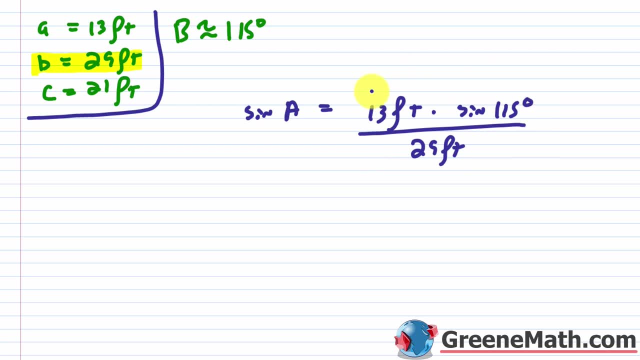 29 feet. Now we're going to end up taking the inverse of this, So you might as well say that A is equal to. let me slide this down: A is equal to the inverse sine of this guy right here. Okay, so let's punch this into the calculator And let me visibly cancel these units And you'll get. 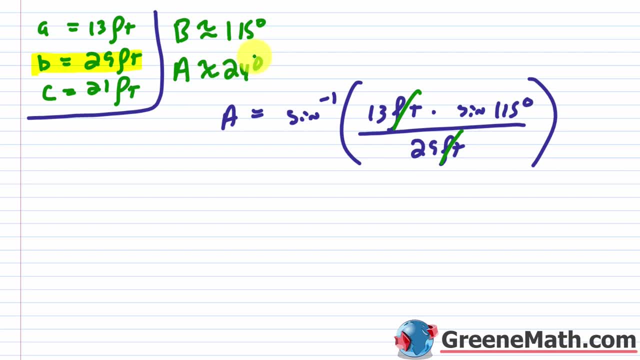 this. So let's go back up and we'll say: B is about 115 degrees, A is about 24 degrees, So let's erase this. And then again for C. all you have to do is do 180 degrees minus 115 degrees minus 24. 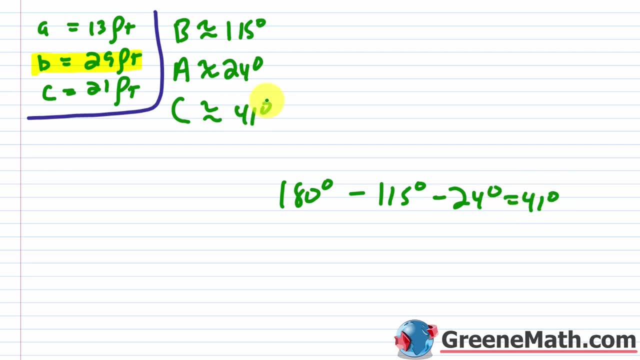 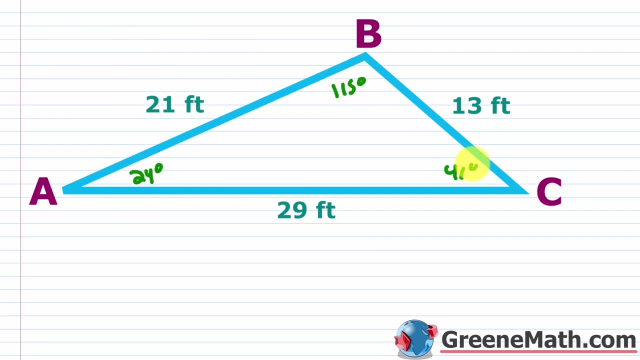 degrees and that's going to give me 41 degrees. Okay, so this is about 41 degrees. So let's go back up and we'll say: B is about 115 degrees, A is about 24 degrees and C is about 41 degrees. 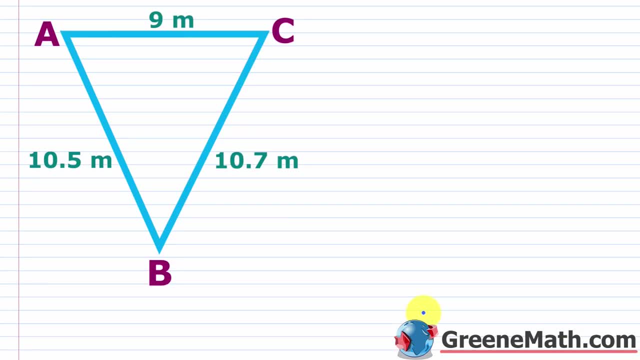 Alright, let's talk about this, Heron's formula and how to find the area of a triangle given the three sides. You can also use this with side, angle side, Okay, and I'll show you that in a moment, But it's much. 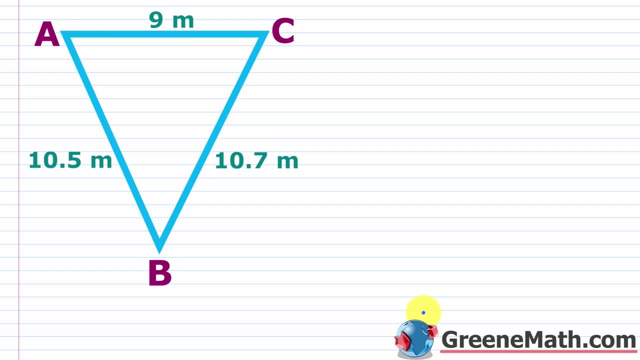 slower than the formula we saw with the law of sines. Okay, So with this guy right here, I'm given that basically, let's say side A is going to be so A is 10.7 meters. Then let's do side B. 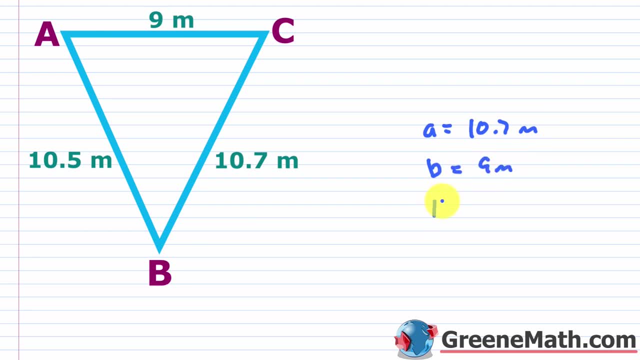 that's going to be nine meters, And then side C is 10.. Let me put the C there, So C is going to be 10.5 meters. Okay, so let me grab this. let's take this away, bring this over here. Let me paste this in here. Okay, let me give you a little. 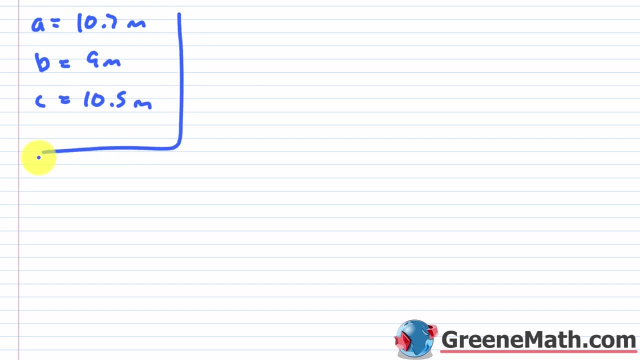 formula. Okay, So for Heron's formula. basically, the first thing is you're going to find the perimeter of the triangle and divide it by two. Okay, in your book you're going to see this called s. So s is equal to. you can say one half times. you sum the sides, So A plus B plus C. 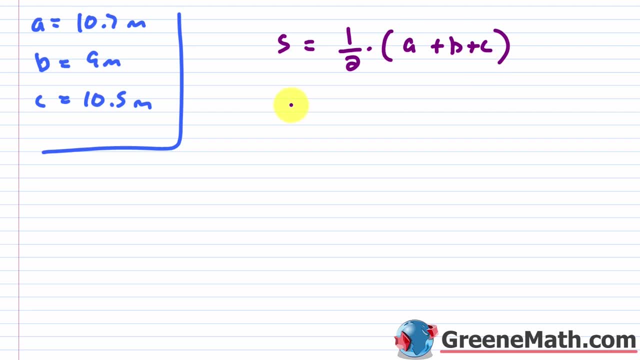 okay, you know how to get the perimeter of a triangle, So in this particular case s would be equal to: we'd have one half times. your a is 10.7. I'm going to leave the units off for now, so 10.7. 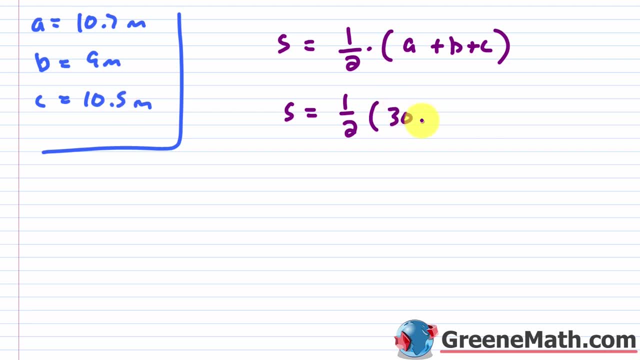 plus 9 plus 10.5 is 30.2. okay, so this would be 30.2. you can put meters in there if you want, it's up to you, and then basically I would divide this by 2, so you could say s is 15.1. okay, so let's say: 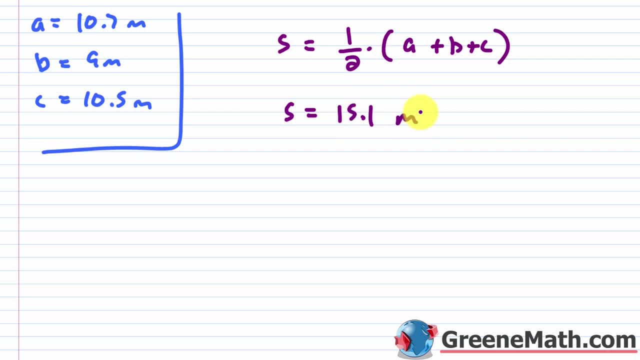 15.1. again, if you want to put meters there, you can. in the end, you know, with area it's whatever units you have squared, okay. so if you want to work with that, that's fine. so then from here, what you're going to do is you're going to plug into this kind of long formula: so the area is equal to. 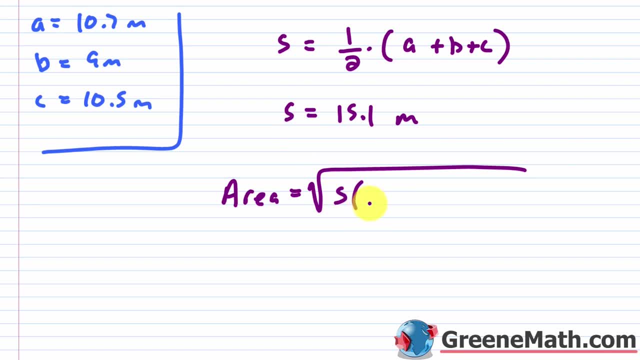 the square root of: you're going to take this s and you're going to multiply it by your s minus your a, then your s minus your b- okay. then your s minus your c- okay. very easy formula to remember. so basically, if I plug in here, I would say: the area is equal to: and again I'm going to leave. 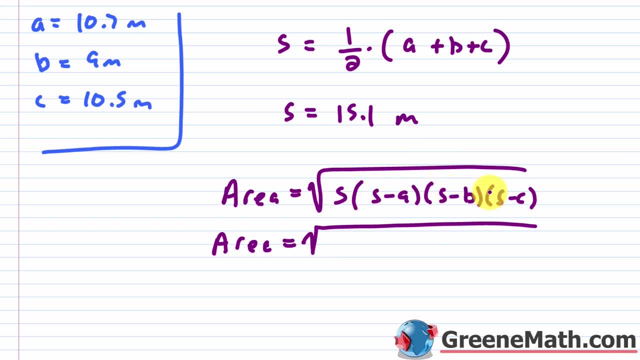 the units off to make this shorter, you would end up with meters, meters, meters, meters, so meters to the fourth power. when you take the square root of the fourth power, you get the second power, or squared, which we know from an area formula. that's what you get. 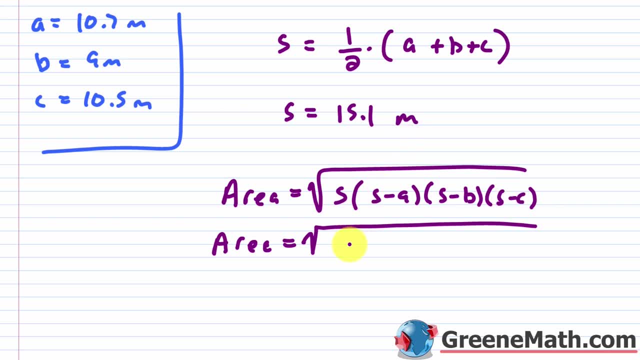 okay, So you're going to end up with meters squared, so I'm just going to tell you that in advance. okay? So basically, for S, this is going to be 15.1, then times, you would do 15.1 minus. 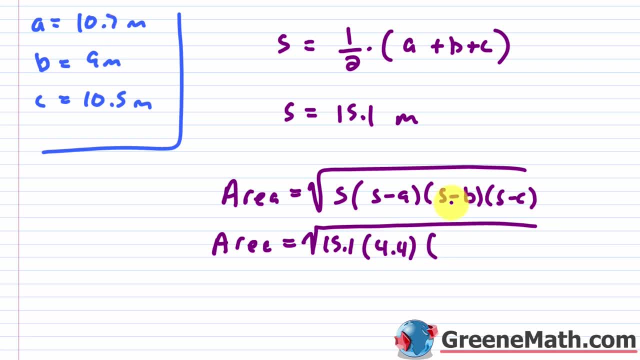 10.7,, which is 4.4, okay, Then S, which is 15.1, minus B, which is 9,, that's going to give me 6.1, okay. And then S, which is 15.1, minus your C, which is 10.5,, which would give me 4.6.. 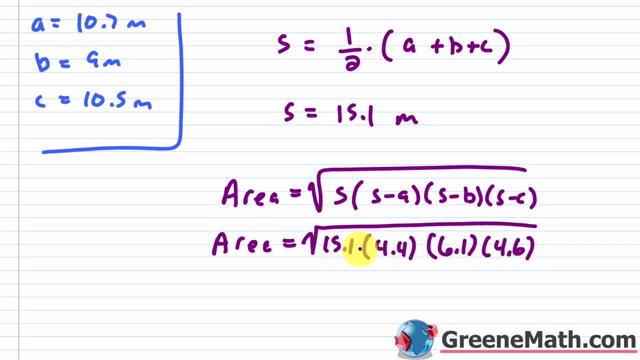 Now, of course, you don't have to set it up this way. you can just punch it straight into the calculator. I just wanted to give you a little insight into what's happening, so I'm just going to crank this out in the calculator and see what I get. So I get about, let's say, 43.2,. 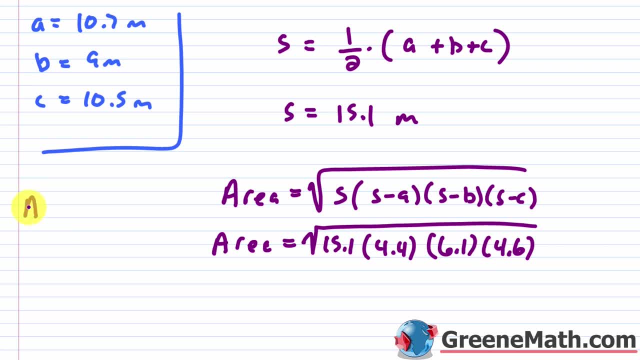 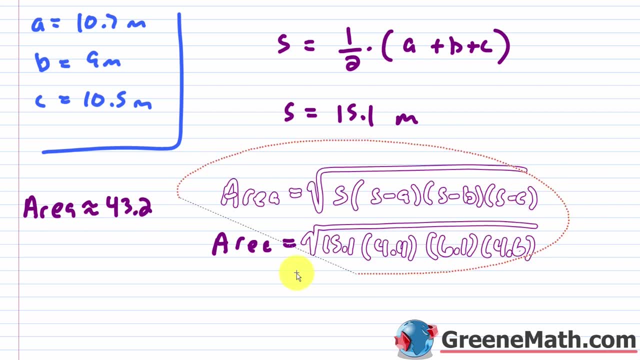 if I round it to the nearest tenth for the area. okay, So I'll say the area of that triangle we'll say is approximately, I'll go 43.2,. okay, Let me slide this down. don't forget your units. you want to put your meters squared because, again, if you had meters, 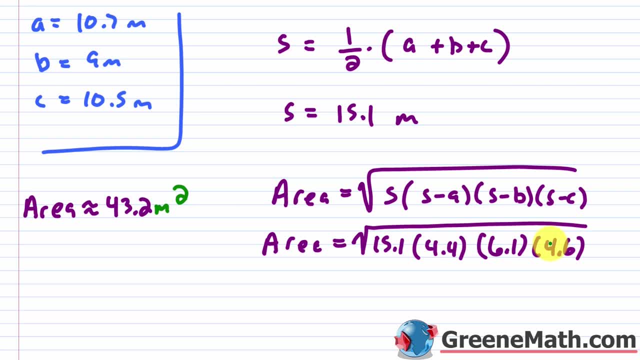 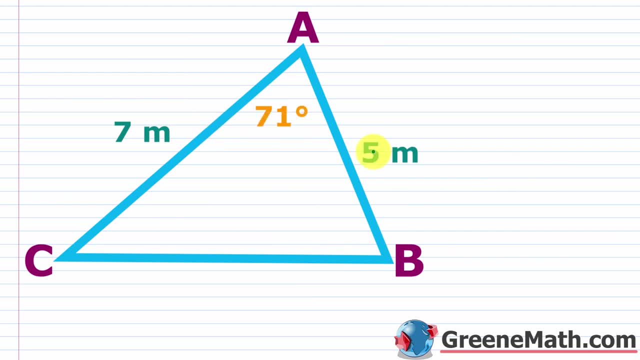 here, here, here and here. okay, you would have had meters to the fourth power. When you take the square root of that, you would have got meters squared, okay. So that's where that comes from. All right, let's look at another example. So this is side angle side here. So, basically, with this, 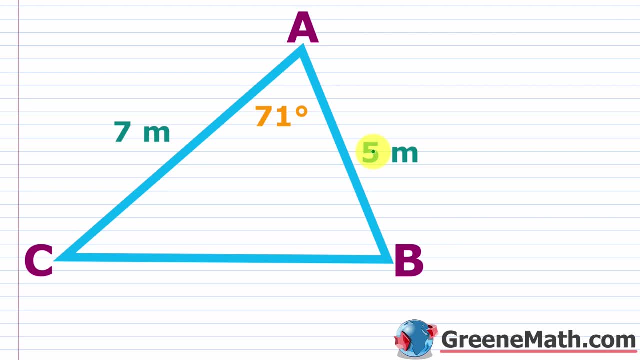 one, it's going to be faster using that area formula with sine. So with that one let me just copy this down. So C, let's say C is 5 meters, we'll say A is 71 degrees and we'll say B is going to be 7 meters. Let me copy this real quick and let me come down here. 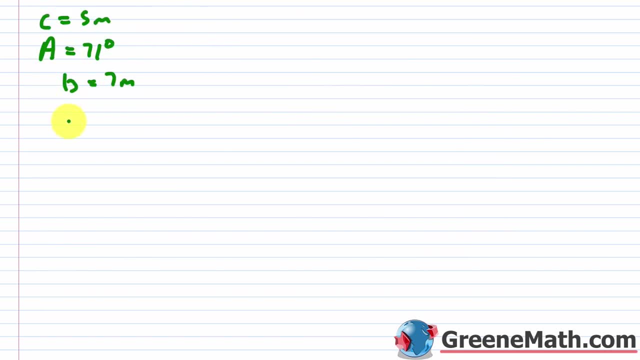 and let me paste this in here, okay. So you remember that formula where we said the area, so the area is equal to one half times. you'll say, in this particular case, I have B and C, so BC, and then times the sine of the angle, that's included, so 71 degrees, So what is B? 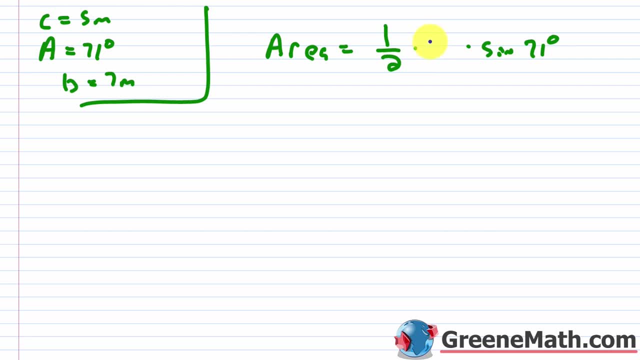 what is C? One is 7 meters and one is 5 meters. So let's just throw this in here, so 7 meters and then 5 meters, and I can't fit this in here, so let me drag this down a little bit. So 7: 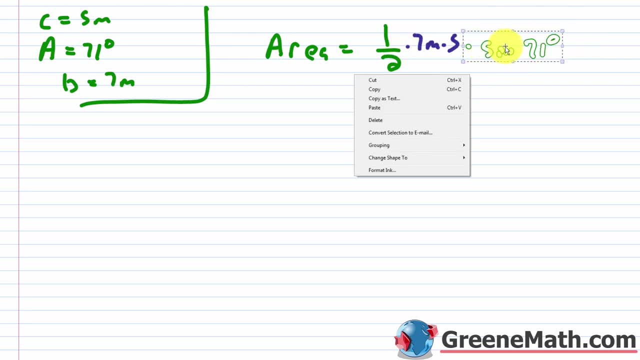 meters and then 5, let me slide this down right there so I can make that fit meters. So basically you'd have what You'd have: 35 meters squared over 2, let me write that like that. so 35 meters squared over 2 times the sine of 71 degrees. Let's punch that into a calculator. 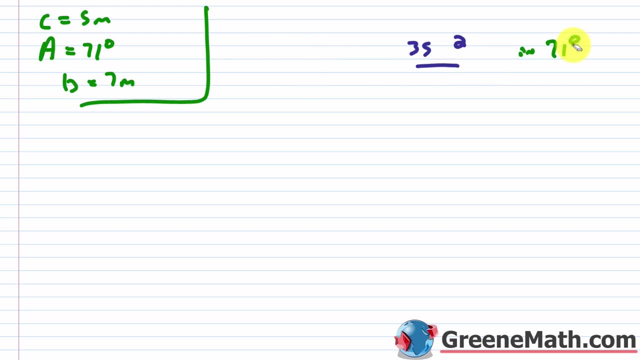 I'll say it's about 16.5 meters squared. So let's say the area. so the area is about 16.5 meters squared. So let's say the area is about 16.5 meters squared. So let's say the area is. 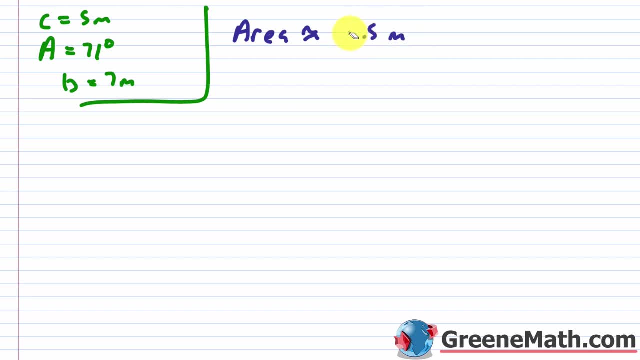 17.5 meters squared. Okay, So we already know how to do it that way. The way I'm about to show you is going to be much slower, but we're going to get a lot of practice. The first thing is, I would 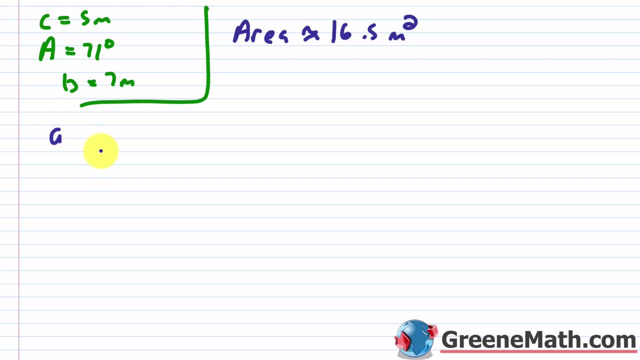 want to find this missing side, lowercase a. Okay, So how do I do that? So a squared is equal to what's not involved here. You have b squared and then plus your c squared and then minus your two times b times c and then times your cosine of the a. Okay, So let's go ahead and say a is equal to. 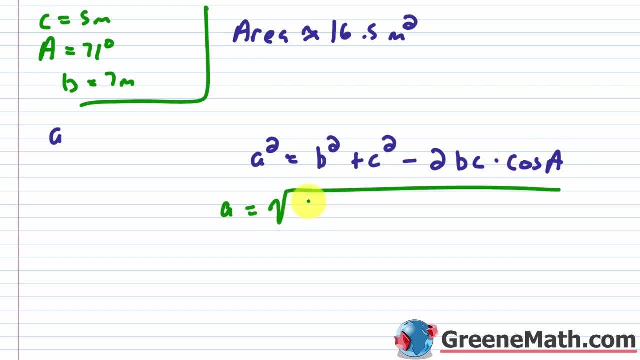 the square root of all this stuff. So b squared is what It's seven. Forget about the units. We'll say it's seven squared plus c squared is five squared minus two times. You're going to have five times seven. Okay, And then let me make that a little bit better, because my handwriting is: 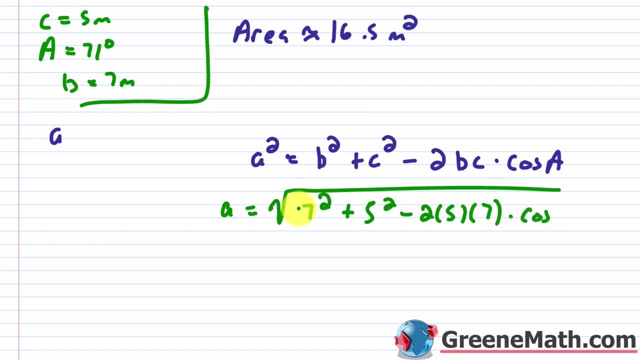 getting pretty sloppy And then times the cosine of this 71 degrees. Let's punch this into a calculator So I get about 7.2.. Okay, But how you round here is really going to matter, because you're going to end up rounding twice. So I'm going to do this. I'm going to do this, I'm going. 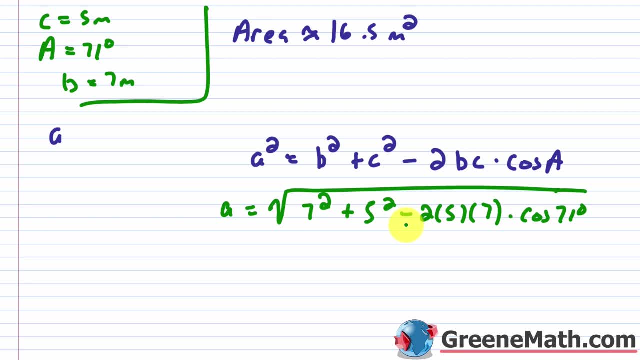 to put 7.2, but that's going to really throw the answer off. So let me put a is about 7.2 meters, Okay. So let's get rid of all this, And then let's quickly use our Heron's formula. So we would say: 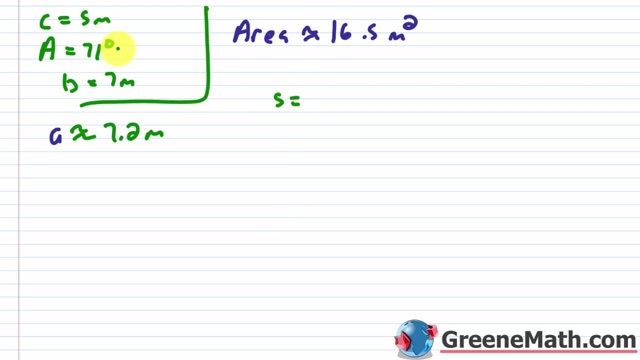 first and foremost, that s is equal to: we would sum the sides, So you'd have five plus seven plus 7.2, which is 19.2 divided by two is 9.6.. And this is going to be in terms of meters. So you can. 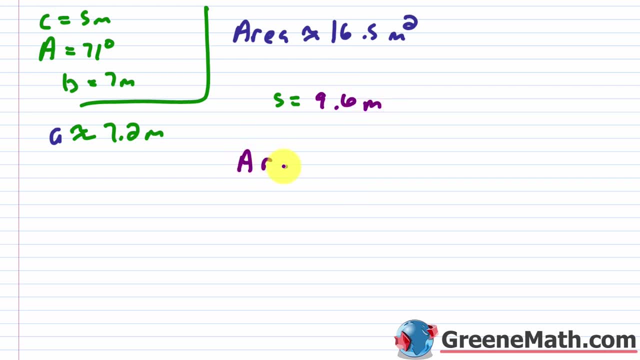 write that And then basically with your area formula, so your area it's going to be equal to 7.2 meters. So you're going to sum the sides, So you'd have five plus seven plus 7.2, again the square root of you. take this guy right here Again, forget the units. So we're 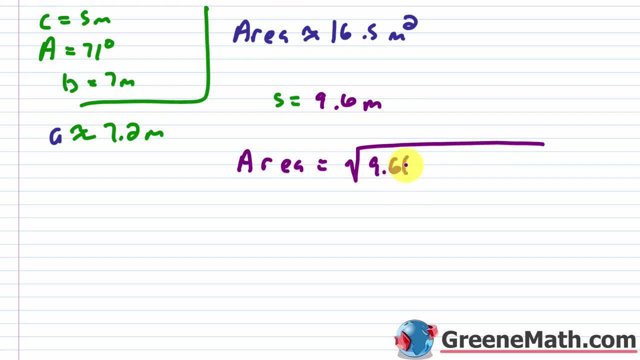 going to put 9.6 times. You would do 9.6 minus, in this case, 7.2,, which is 2.4. And then you'd have times: you do 9.6 minus your seven, which is going to be 2.6.. And then you would do 9.6. 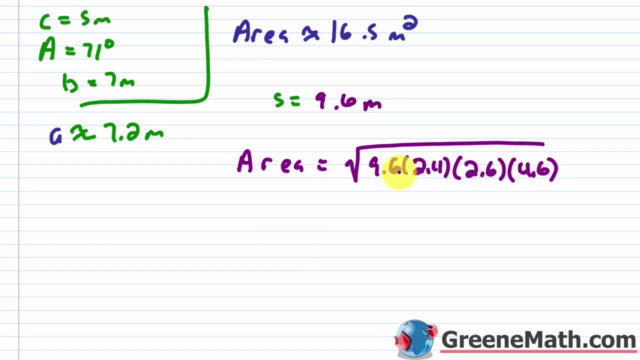 minus your five, which would be 4.6.. Punch this into the calculator and you'll get. your area is approximately, I would say about 16.6.. 16.6 meters squared here. So you can see there is a difference based on the rounding. Okay, Here. 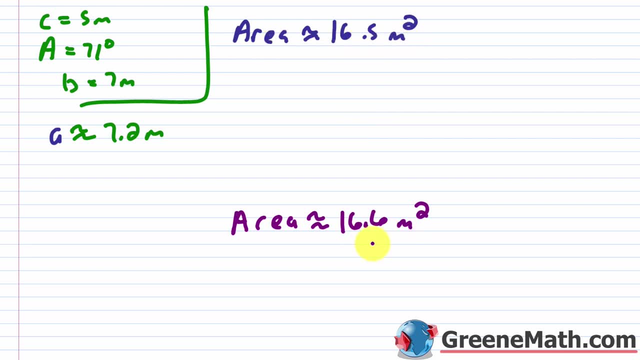 with the better formula. we got 16.5 meters squared here because we ended up rounding twice. We got 16.6 meters squared. So again, if you get side, angle, side, you want to use that first formula. I'm just showing you can do it this way If you get this on a test sometimes. 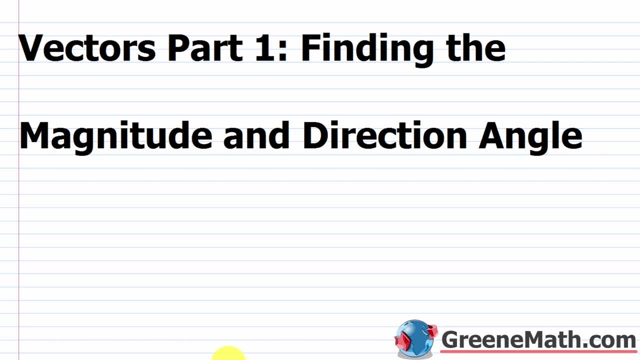 they want you to do that, just to get some extra practice. In this lesson we want to give an introduction to vectors And specifically here we'll focus on finding the magnitude and also the direction. So we're going to do that, So we're going to do that, And then we're going to 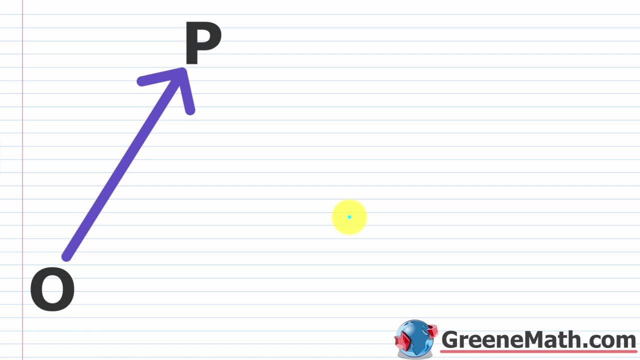 look at the direction angle. All right, So when we work with vectors, we're basically going to see this as a directed line segment. Okay, So this is going to have what we call a magnitude or a length, and then also a direction, which is given by the arrowhead. Okay, So if I look at this directed 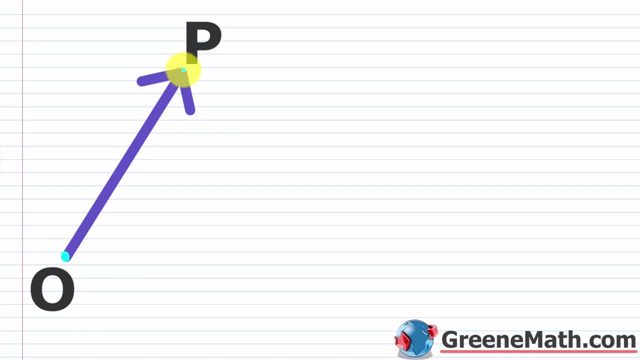 line segment with an initial point of O and a terminal point of P. you can see that it has a magnitude or a length, Okay, And it also has a direction given by, again, the arrowhead. Now, the way you would notate this would vary by textbook, but I would take my initial point here. 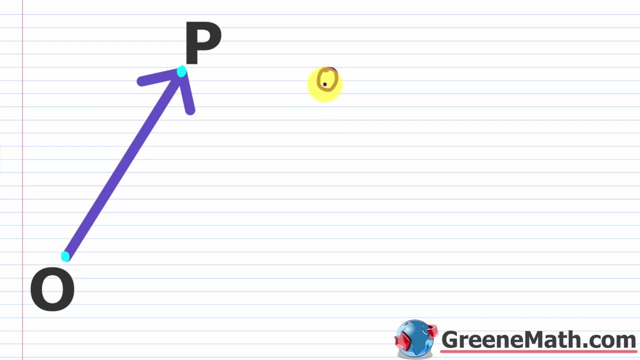 of O: Okay, And I would list that first. That tells me it's the initial point. Then I would take my terminal point P and I would list that second. Okay, That tells me that's the terminal point. So the order here, when you're using two letters is going to matter, Okay, And then I want 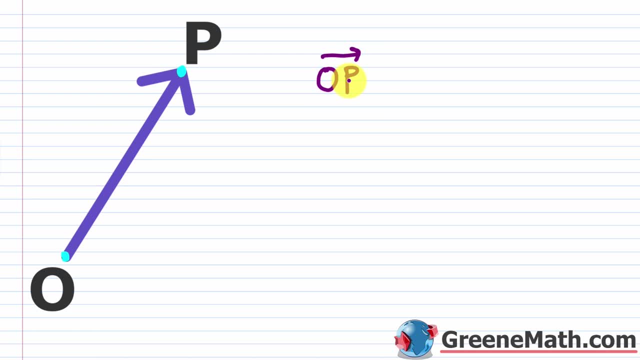 to put a little arrow on top. Okay, So this is the typical way that you will see this. notate. Now you could also use a lowercase letter. Okay, Something like. let's say V. Okay, Something like, and do the same thing. Right, But this one is going to give you the information about Hey. 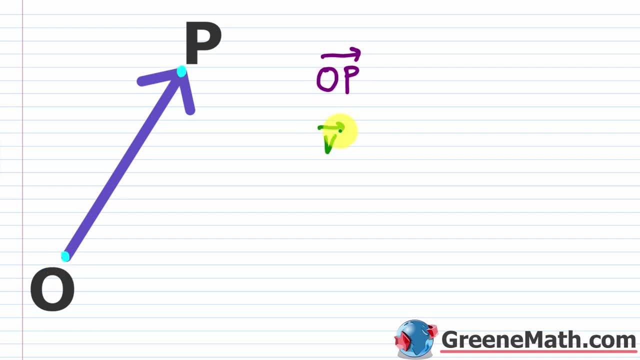 O is the initial point and P is the terminal point. This guy just tells you you have a vector. Okay, Now let's erase this for a moment. I want to show you a few other ways that you might see this notated. So in your book you might see this: Okay, Where they just put that guy like that. 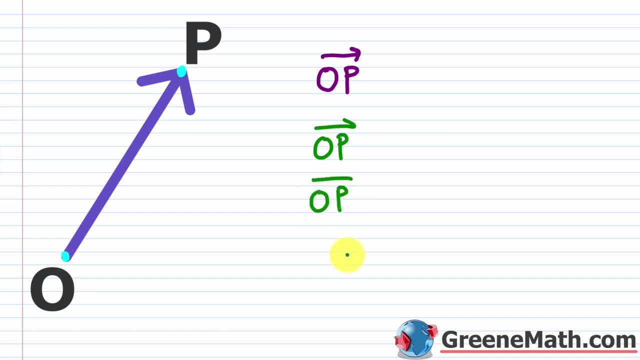 Okay, You also might see this listed with a bar on top, And then, lastly, you might see them just use a boldface font. Okay, So you might see them just do that. Now I'm going to stick with this tutorial. In a few minutes I'm going to start talking about the magnitude or the length of this. 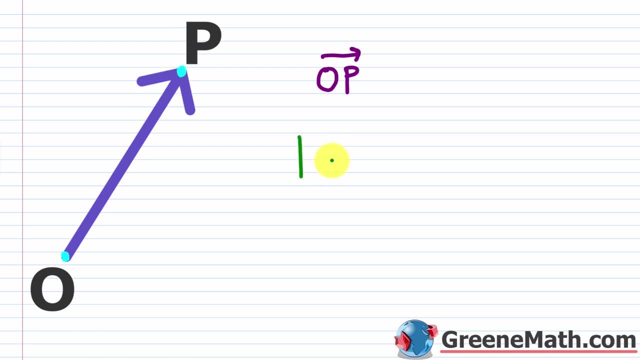 guy: Okay, And the notation for that is basically where we're going to use these vertical bars. So the magnitude of this vector OP, I could put it in vertical bars to show that. or sometimes the textbook will use two. Okay, Two vertical bars Okay, So go with whatever. 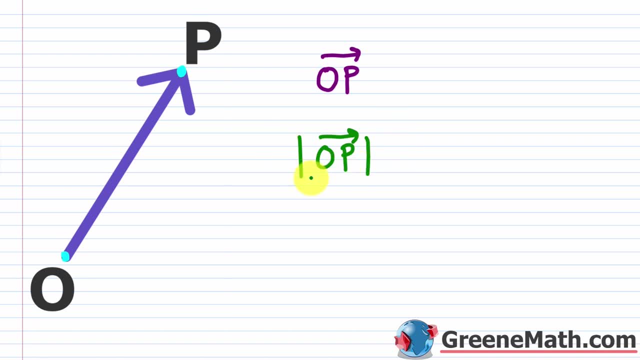 your textbook goes with. I'm going to use single bars here, because that's what my textbook uses. Now, if we look at these two directed line segments, or these two vectors, the first thing is if I'm using the two capital letters to name them. 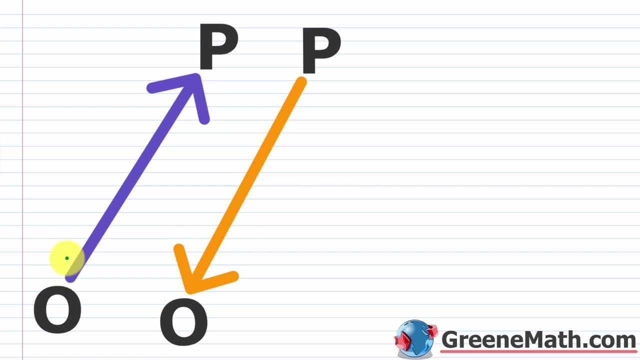 this guy would be named OP. Okay, That vector OP. Here is going to be your initial point And here's going to be your terminal point, Right? So this guy would be the vector OP, like this. Now, this guy is not going to be the vector OP, Okay, Because the initial point is here now And the terminal 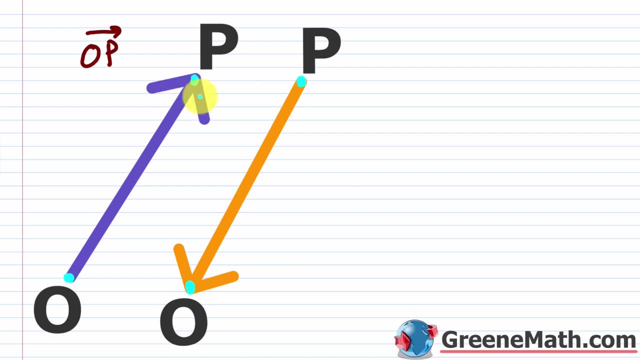 point is here, right, These have different directions. Look at the way the arrowheads are facing. Okay, This one is facing this way. This one is facing this way. Okay. So, different direction, same magnitude, But this one is going to be called PO, So this: 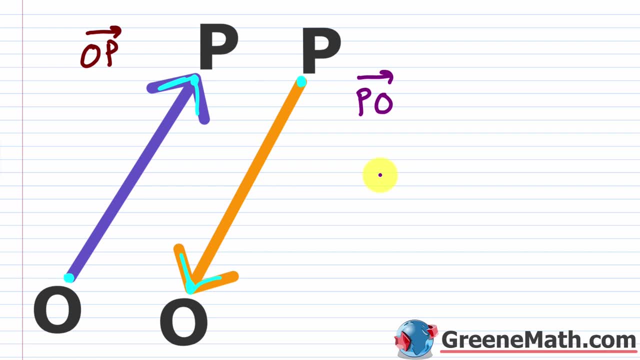 will be vector PO. Okay, Let me get rid of this and make that a little bit better. Now I can say right here that this vector OP is not equal to this vector PO, And the reason they're not equal is because for two vectors to be equal they have to have the same magnitude. 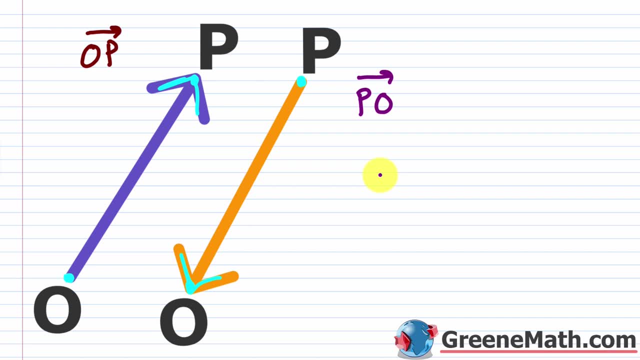 or the same length, And also they have to have the same direction. These do not have the same direction, even though they do have the same length. So I can say this vector OP is equal to this vector PO. All right, So now let's think a little bit about the magnitude. 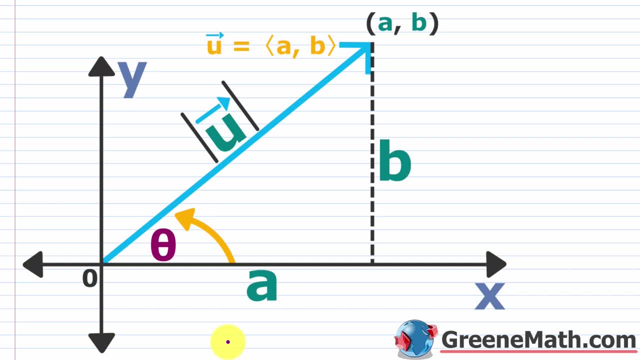 and how we find that. Also something called the direction angle, and then the component form. Okay, So let me start with the component form, because I think everything kind of builds off that. So, first and foremost, you see on this sketch, the way this is drawn, we have 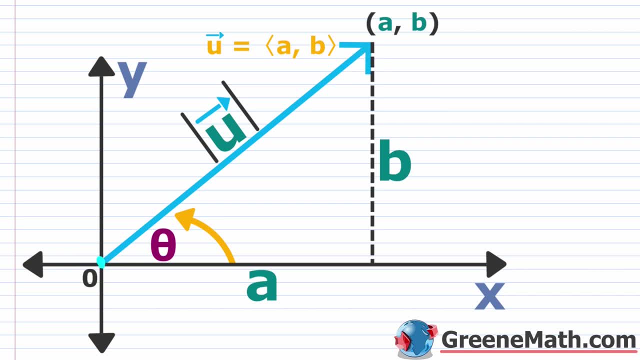 our initial point at zero comma zero or the origin. Okay, So let me label this: This is zero comma zero. Then we have our terminal point. our terminal point at this A comma B. Okay, This guy has an initial point at zero comma zero. We call this a position vector, Okay. 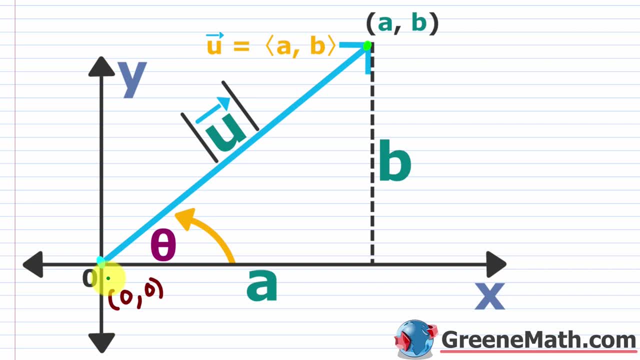 Or we say it's in standard position. Now, when you have a position vector, or when it's in standard position, you can just list the coordinates for the terminal point. That's all you need, because you know the initial point is at the origin. Okay, You don't need any more information. 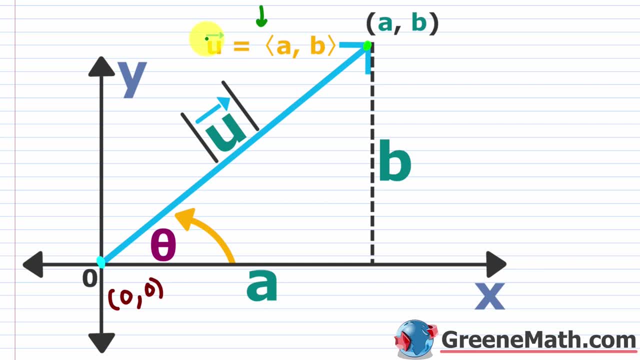 So the way we list this is called component form. Okay, So here I've named my vector U, So the vector U is equal to. you'll see, we have these angle brackets here and we're just at the A and the B. all this is is the X and the Y from the ordered pair we're just listing. 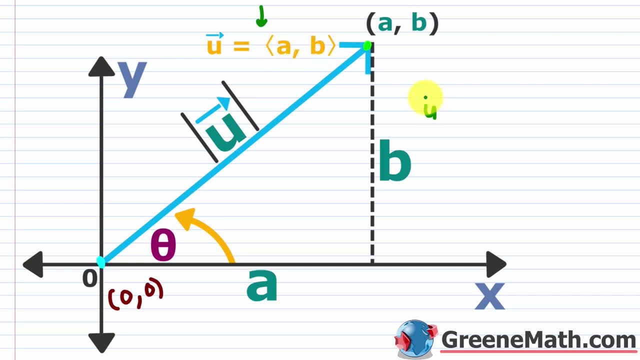 it inside of those angle brackets. So if I said that I had a vector, U is equal to, let's say, I had three comma four. Well, I know I didn't make those brackets very well. I know that the X location is three and the Y location is four. in terms of the point, 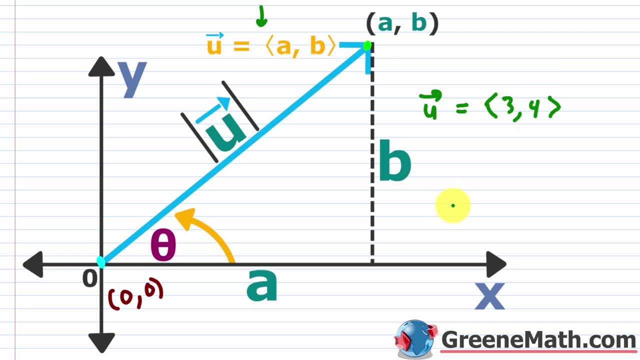 Okay, The terminal point for that vector. So I would start with the initial point at zero comma zero, and then I would draw a terminal point at three comma four. I would just draw line segment. That's all I'm doing. Okay. So additionally, we also have something called. 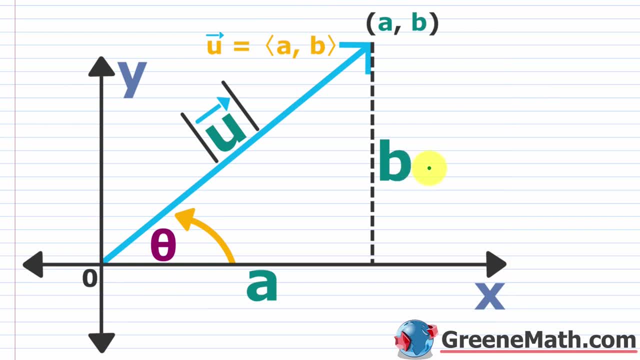 let me just erase all this. We don't need this anymore. We also have something called the magnitude of the vector, which we already talked about. It's the length of this guy, right? So if I said what is the length of this guy, right here. So if I just drew this line right here, 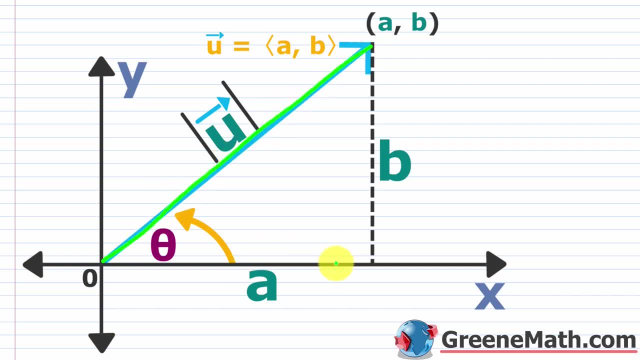 what is the length of that? Well, again, normally if we form a right triangle, okay, we can do this with the distance formula. Let me just call this side C for a moment. So I'll say C, which is the hypotenuse typically. Okay. So C, I'll say C squared is equal to this: A squared plus B squared. 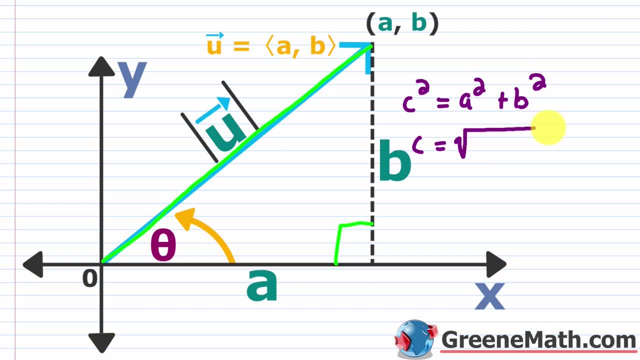 So we know, if we want C, by itself, we say C is equal to the principal square root. We don't need the negative one of A squared plus B squared. Okay, Well, now instead of C I just have the magnitude of U. So I'm just going to replace that. Okay, That's all I'm doing. So the magnitude. 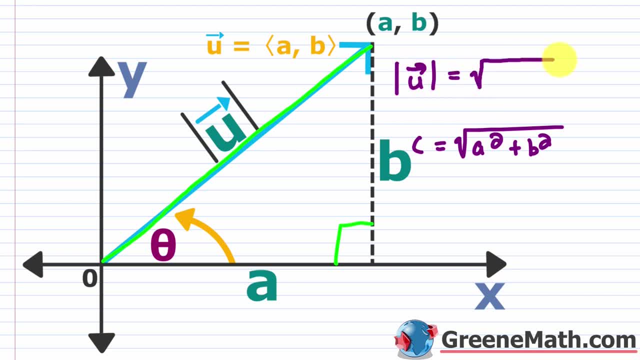 the magnitude of U is just equal to the square root of A squared plus B squared. Now, in the case where you're not given a position vector, okay, you're going to either have to put it into component form or use your original distance formula, right, Remember, the distance is equal to you have this square root. 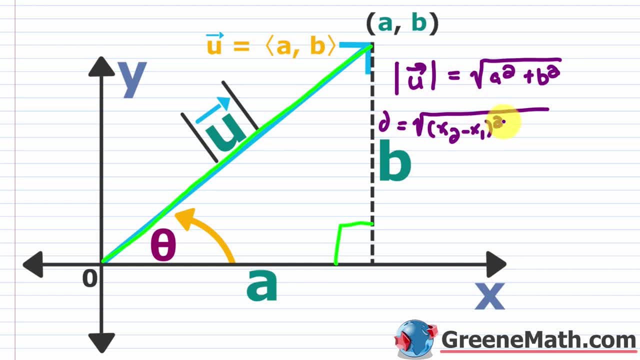 of you have the quantity X sub two minus X sub one squared, plus the quantity Y sub two minus Y sub one squared. Okay, In this particular case, your point down here is zero, comma zero. So if you do this it just becomes A. this is going to be A right For the X location: A minus zero. 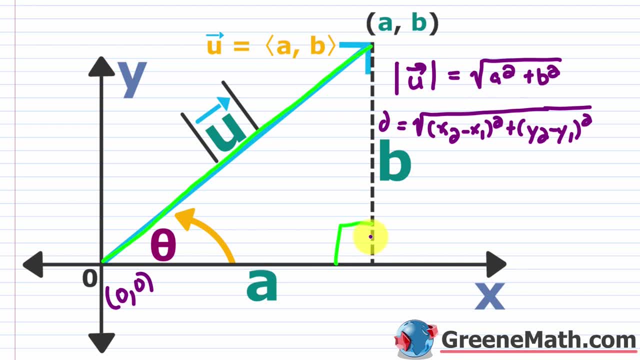 which is A being squared, Then plus this would be B minus zero. Okay, So it would be B just being squared, Okay, So that's all it is. So let's get rid of this and we see how to find the magnitude. Now let's talk about how to find the direction, angle, because 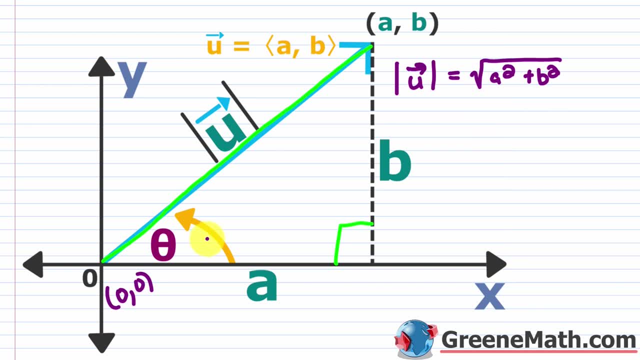 this one's quite confusing, Okay. So basically, the direction angle is going to be this positive angle theta here between the X axis, Okay, And our position vector. Now it turns out that it's pretty easy to find this overall, Okay. All you really need to do is some basic trigonometry. 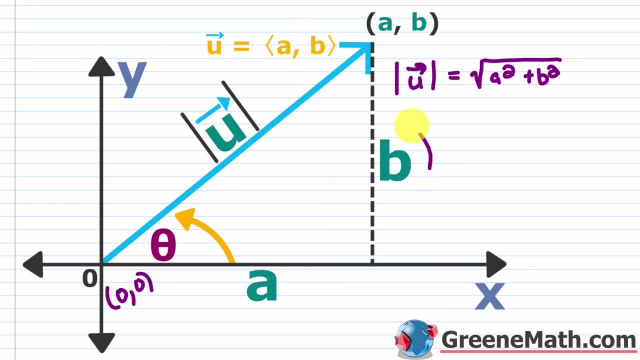 in these problems, If you're given A and you're given B, So if you're given this and you're given this and you're trying to find this angle here, what can you do? Well, remember, the tangent is Y over X. Okay, In this case it would be B over A. So the tangent 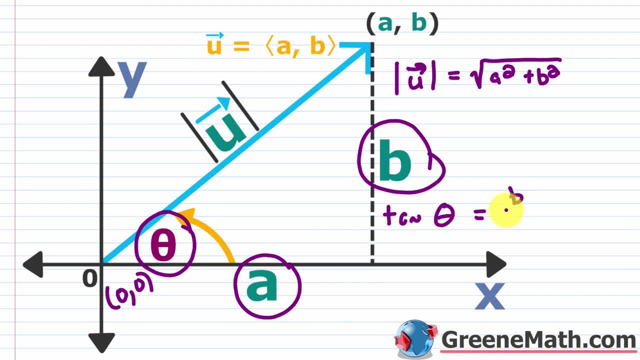 okay, of this angle, theta is going to be equal to B over A And you could say specifically, where A does not equal zero, Okay. But you're going to have to do more work than this because, again, if you involve the inverse tangent function, remember that guy is going to only return. 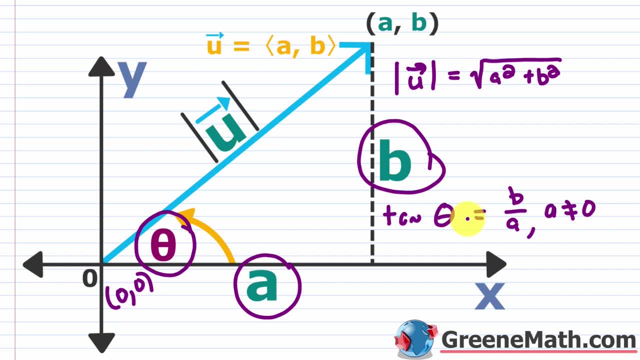 something from quadrants one or four. Okay, So you have to basically think about this by getting a reference angle in most cases and then figure out what quadrants you're in. So you're going to have to do a bit of detective work. Okay, Let's go ahead and take a. 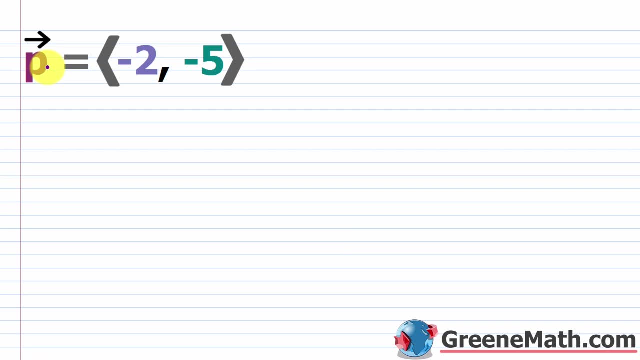 look at a simple problem. So I'm given a vector P, Okay, And the component form gives me a horizontal component of negative two and a vertical component of negative five, Okay. So if you wanted to sketch this guy, you would have one point at the origin, Okay, At zero, comma zero. Okay, That's your. 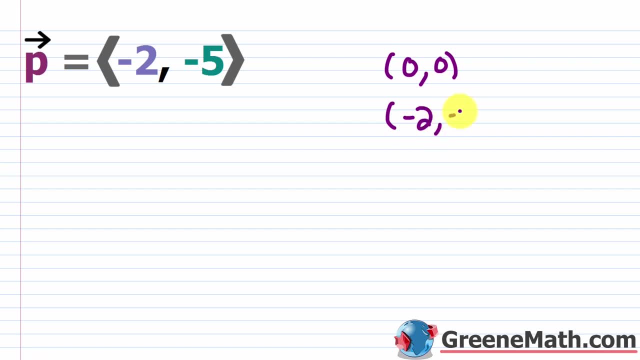 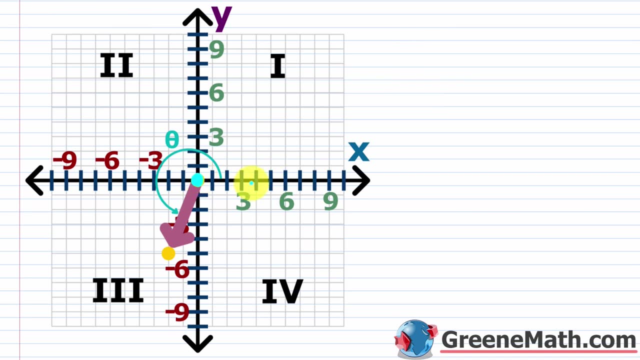 initial point And then you'd have a terminal point at negative two comma negative five. Let's just look at the graph real quick. So you see your initial point is here at zero comma zero, Okay, And your terminal point. you're going two units to the left and five units down. 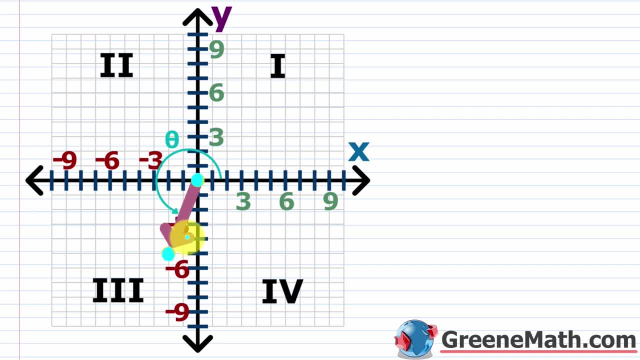 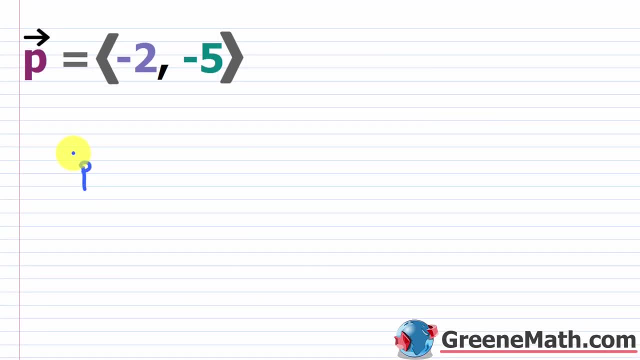 So it's at negative two comma, negative five. Okay, It's just a directed line segment, That's all it is. So if we think about the magnitude of this guy, again, that's pretty simple. The magnitude of this vector P is going to be equal to the square root of- again, you're going to square. 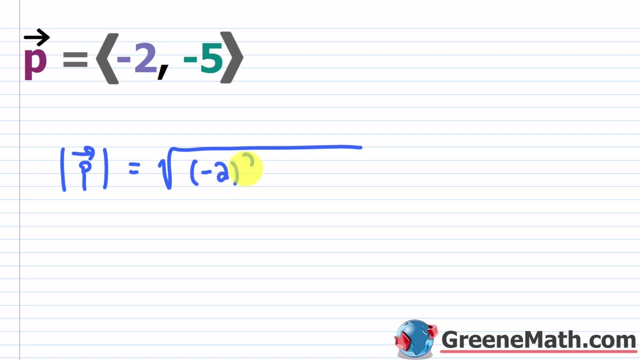 each one and then sum the results. So I'd have negative two squared- Okay- Make sure you put in parentheses- Then plus you'd have negative two squared- Okay. So you'd have negative two squared. Negative five squared- Okay. So you want the negative and the five being squared and the 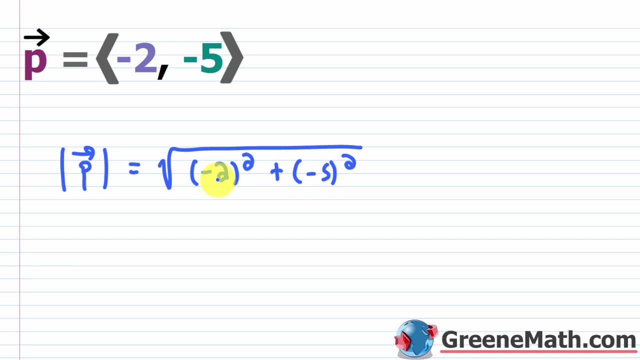 negative and the two being squared, Make sure you use parentheses. Okay. So what I'm going to do here is I'm going to say that the magnitude of this vector P is going to be equal to the square root of. let's go ahead and say negative. two squared is four, Okay, Plus if you do negative. 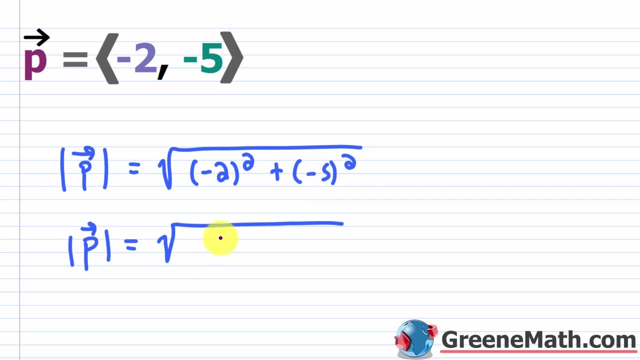 five squared, that's 25.. So that would be four plus 25 or 29.. Okay, So this is the magnitude of this vector P. Okay, Nothing more than just the distance formula. Now, if we think about the direction angle, this is where things get a little bit more tricky. 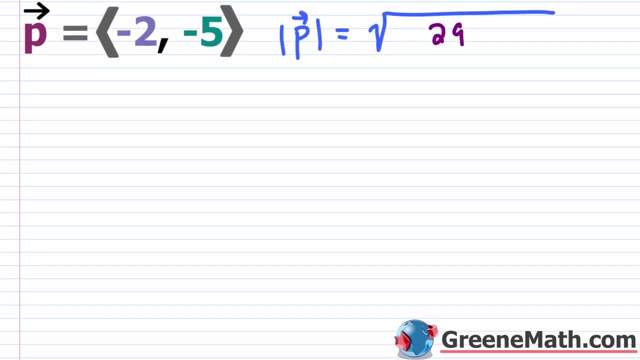 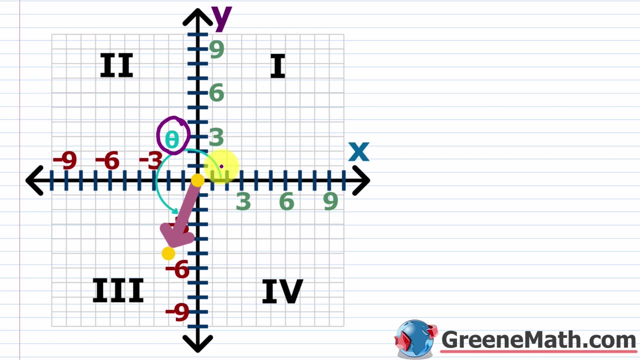 Let me get this out of the way. Okay, If I go back, I want you to observe a few things and I can just erase this. We're trying to find this angle theta here. Okay, If we think about this, if we swing this around, we see that this guy is in quadrant three. Okay, So in quadrant three. 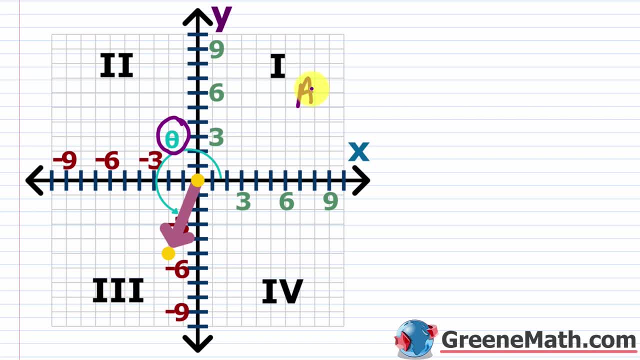 if we think about tangent, it's going to be positive, right? Remember this. all students take calculus, Okay, But if I use my inverse tangent function, I'm not going to get something in quadrant three, I'm going to get something in quadrant one. So if I go back and I 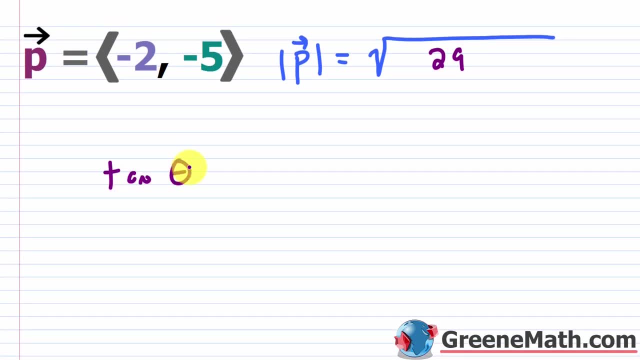 think about this guy. remember that tangent of theta is equal to you. take your Y value or your vertical component, which is negative five over you, take your X value or your horizontal component, which is negative two, And so basically I could say the tangent of theta is really equal to five. 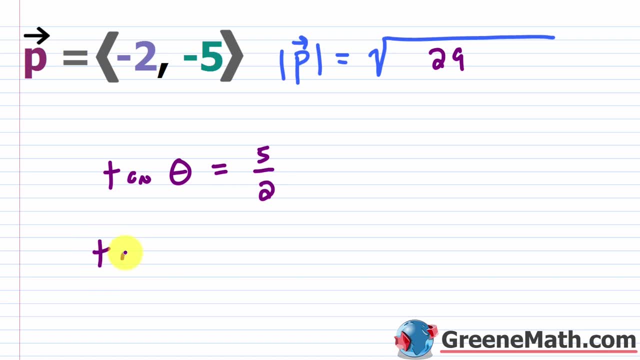 halves, right? So if you do the inverse tangent on this, so you do tangent inverse of this five halves, you're going to get something. let's say it's approximately, I'll go with 68.2 degrees. Okay, So 68.2 degrees, And again, I'm just rounding. So if I know that this guy right here is the 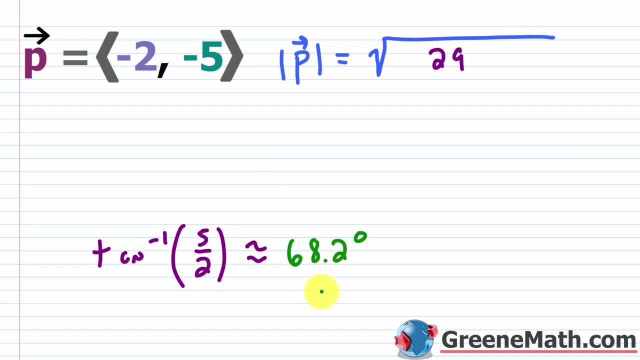 result of the inverse tangent function. well, again, if I'm in quadrant three, this is not my angle, Okay. So people mess up all the time and say, okay, well, theta is going to be 68.2 degrees. 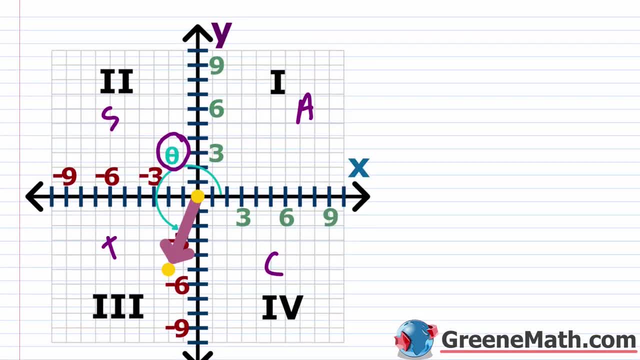 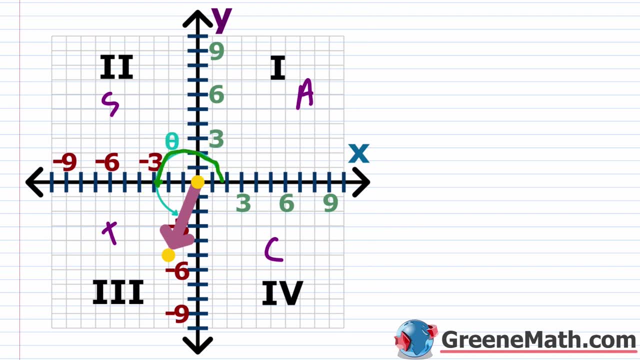 That's wrong, because I'm in quadrant three, So if I go back, you can visualize what's going to have to happen here. Okay, I've got to go 180 degrees first, Okay, And then I also need to add on top of that that reference angle to get. 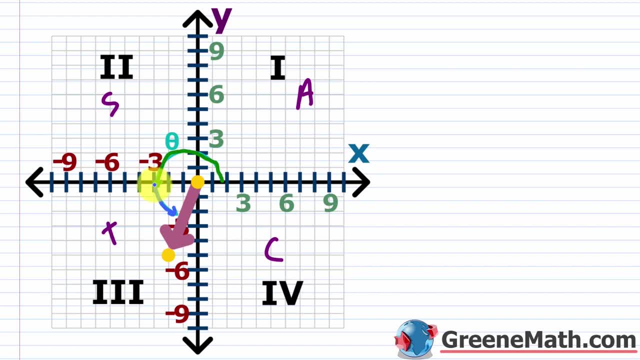 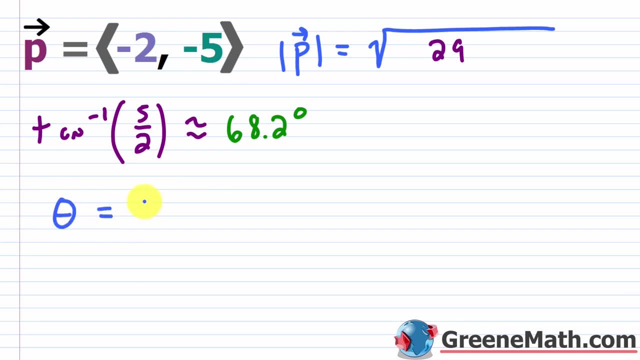 the rest of the way. Okay, So I need 180 degrees plus the reference angle to get this angle here, theta. So if I go back, all I want to do is say theta is going to be equal to 180 degrees plus 68.2 degrees, And you can put approximately here. Let's just leave the equals for a moment, I'll 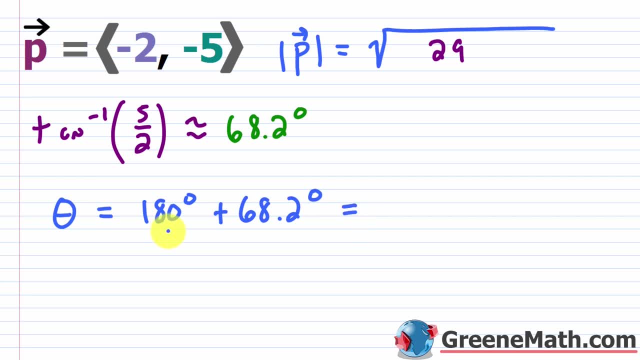 just go ahead and change it in the end. So this is going to be what it's going to be: 248, 248.2 degrees, And then I'm going to add on top of that that reference angle to get the rest of the. 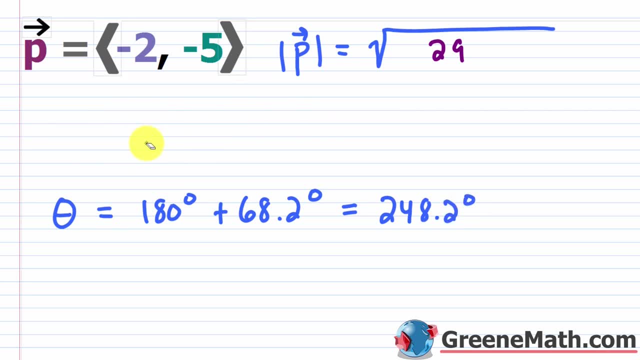 way. Okay, So that's our direction angle. It can be a little bit confusing. Just make sure you understand what quadrants you're going to be in and that when you're working with the inverse tangent function, you're getting something in quadrant one or four only. Okay, So let's go. 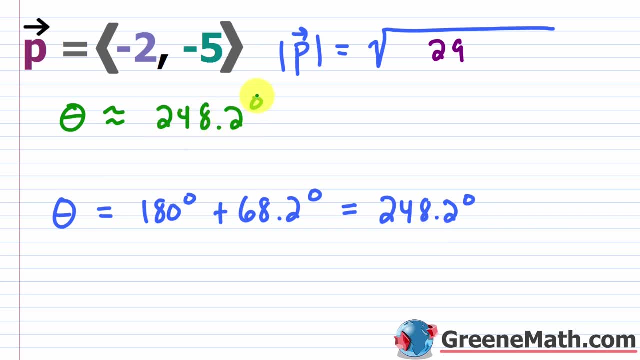 ahead and put this as 248.2 degrees, Okay. Also, I should note that if you get something in quadrant four from the inverse tangent function, remember it rotates clockwise to get that. Okay, So that's going to be your angle either. Okay, So you got to do a lot of detective work when you're doing 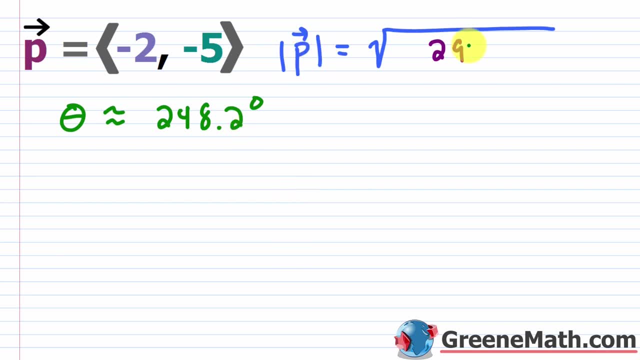 these, Okay. So we found that the magnitude of our vector P is a square root of 29 and the direction angle is approximately 248.2 degrees. All right, Let's look at another easy one, And then I'll show you something that's a little bit harder. So we have this vector V here, Okay, And the horizontal. 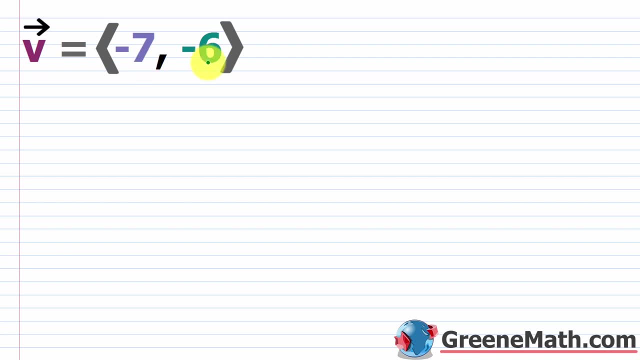 component is negative seven. The vertical component is negative six. So again, if I wanted to find the magnitude, so the magnitude of this vector V, this is equal to the square root of. you could say: negative seven squared, Negative seven squared, plus negative six squared. Okay, Like this. So the magnitude of this vector V. 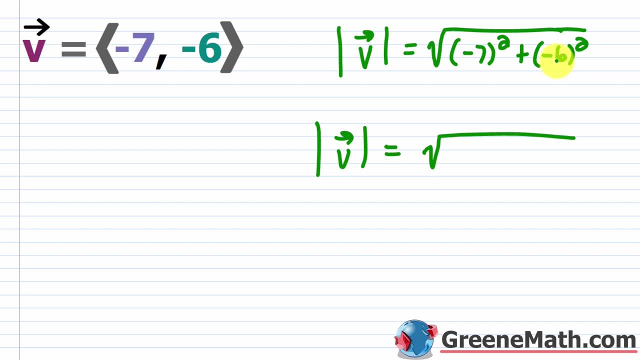 is equal to. let's go ahead and say: this is 49 plus 36.. So that's going to be 85 in here. So basically the square root of 85. really can't do anything to simplify that, So that's just going to. 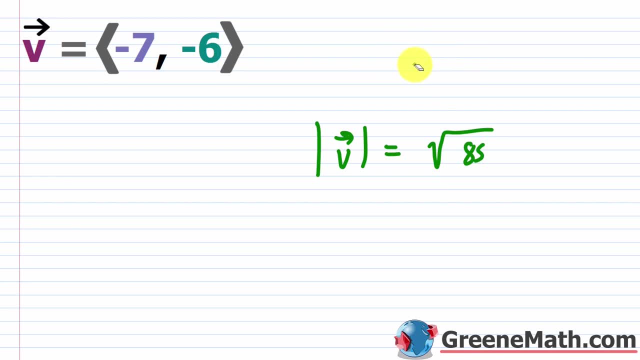 be our answer. Okay, Let's get rid of this and let's just drag this up here And again. finding the direction angle usually takes a little bit longer because you got to plug some stuff in. Now, if I think about this again, the tangent of theta. 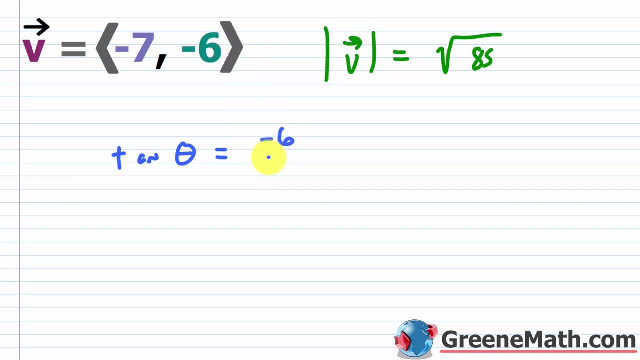 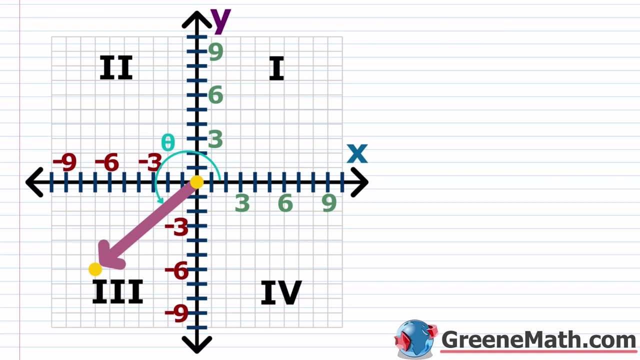 I'm going to end up with something in quadrant one. Where is this guy at? If I graph it again, my initial point is here at zero comma zero, My terminal point. I go seven units to the left and six units down, So it's at negative seven comma negative six. Okay, So if I look at this, 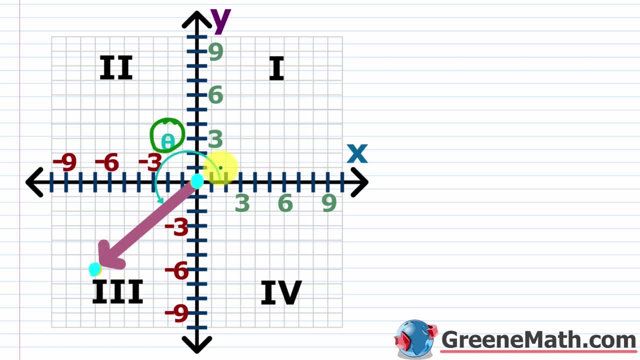 guy, I'm going to be in quadrant three right. So I'm going to be in quadrant two, So I'm going to be in quadrant three right. This is the angle theta that I'm trying to find, So I've got to. 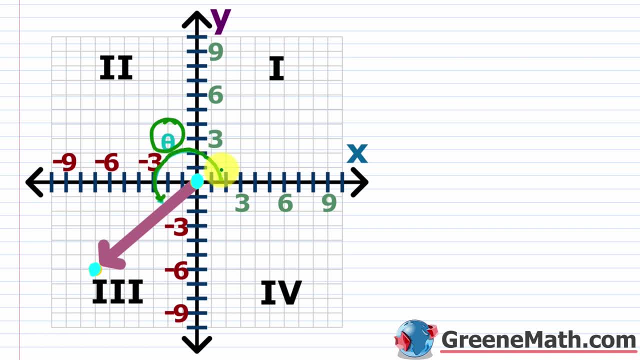 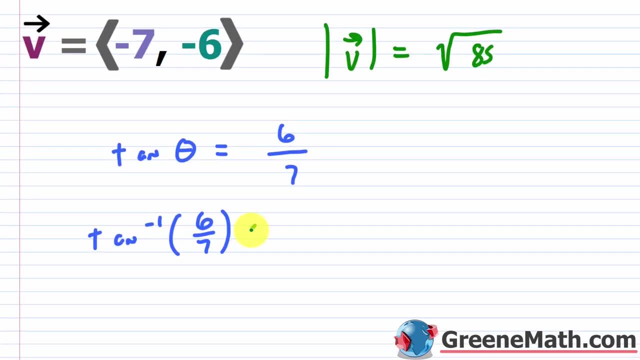 swing all the way around here. So remember what we have to do. We've got to go 180 degrees and then plus that reference angle to get there. So let's go back and let's punch this into the calculator And that's going to give us about 40.6 degrees, Okay. So again, when you think about 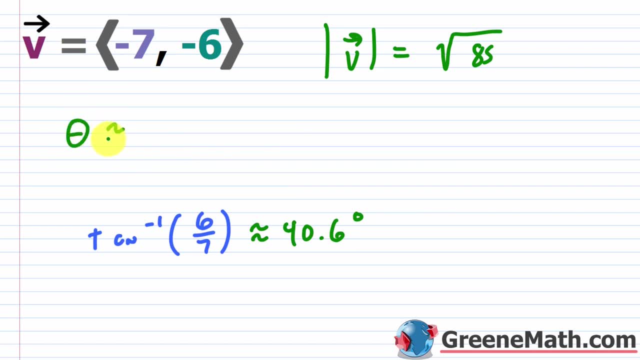 this. I'm going to say that my direction, angle, theta, I'll just put approximately here: I'll go 180 degrees plus I'll go 40.6 degrees, Okay, So what is this going to do? I'm going to say that. 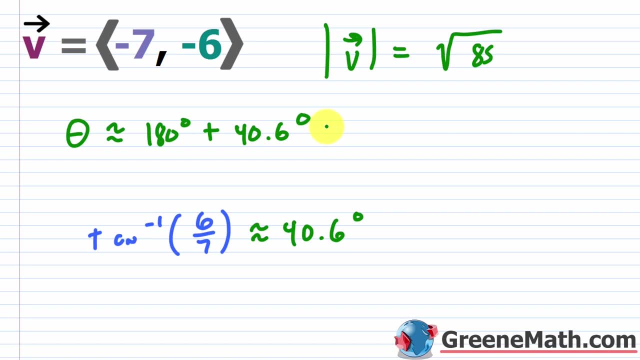 it's going to give me 220.6 degrees. So let me erase all of this and let's just put our answer here. So 220.6 degrees. So again, the magnitude of this vector V is square root of 85.. The direction: 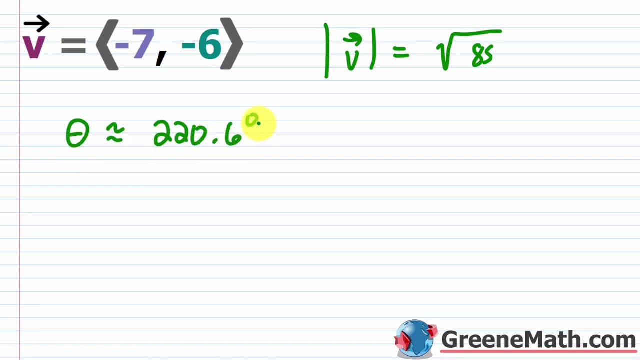 angle is approximately 220.6 degrees. All right, let's take a look at another example. So this one involves a little bit more work. So we have this vector PQ. Okay, So we know, because of the way we said, that the first letter here, P, is the initial point, right? So the coordinates are. 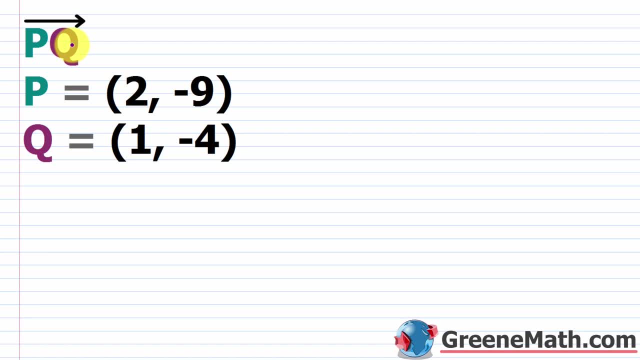 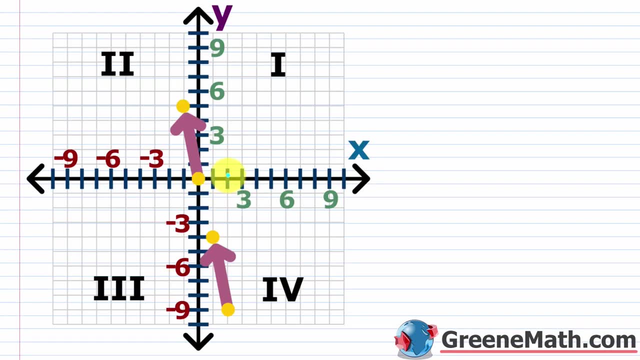 two common negative nine. The second letter Q is the terminal point. So the coordinates: one common negative four. Okay, Let's go ahead and sketch this real quick. So if we look at this guy, we go two units to the right and nine units down. So that's right here. This is going to be your P. 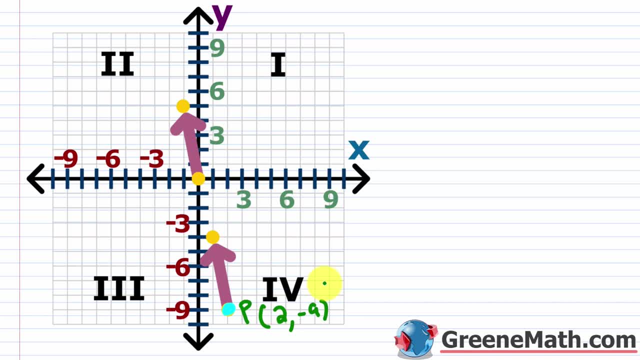 or your initial point. Again, this is two common negative nine, And then the other one. here, if we go one unit to the right and four units down, we're going to be right there. So that's our terminal point. So again, this is one common negative four. So the first thing you want to do, 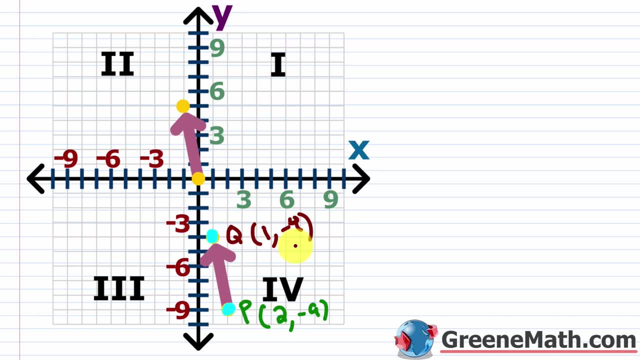 if you have a problem like this, you want to put it in the component form Again, this is where the coordinates for the terminal point are given only because the initial point is at zero comma zero or the origin. Okay, So you'll see that I already have this graph right. So this is zero comma zero. 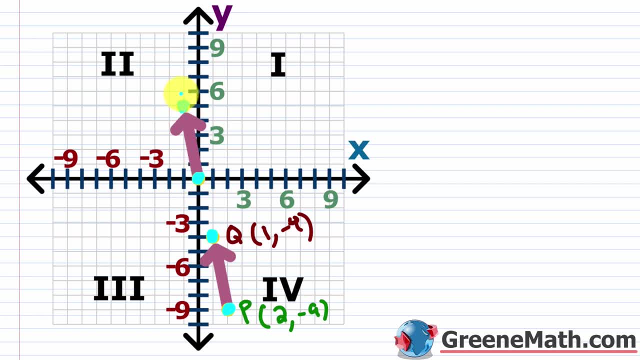 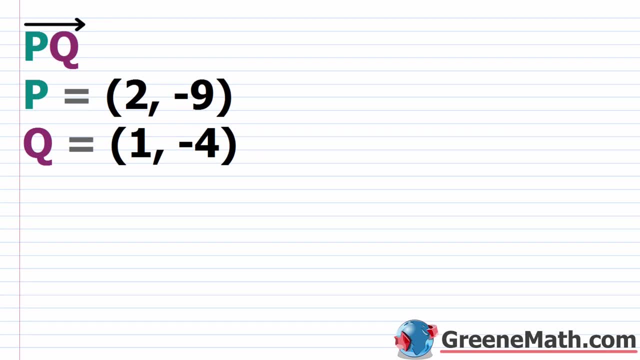 or the initial point, And then you'll see the terminal point is at negative one comma five. So where does this come from? How did I get that? Well, if you go back here, it's a simple little formula, All you really want to do. let me come over here. 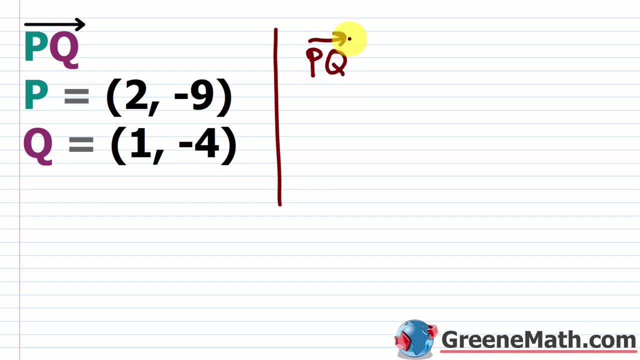 and say: for this vector, PQ, Okay. And sometimes books will rename this with a lowercase letter Once it's in component form. that's up to you. if you want to do that, Okay, I'm going to keep it as it is. So I'm going to say: this is equal to. I'm going to put my little angle brackets there. 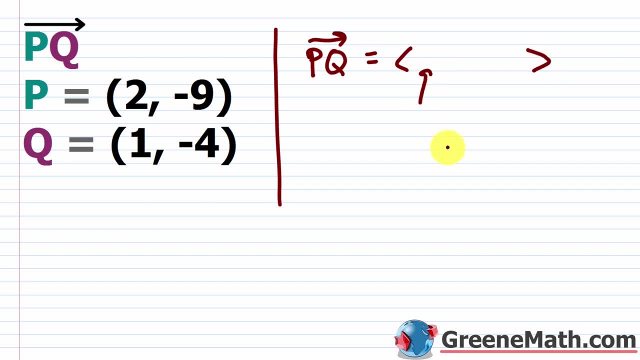 And basically to get this position here, you go with the X value from your terminal point. Okay, So I'm going to take this one right here, Okay, And then I'm going to subtract away the X value. Okay, So one minus two gives us negative one. Now you want to go in that order. I know, sometimes 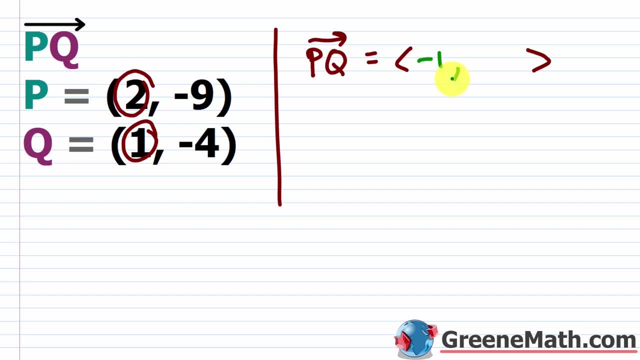 when you work with these formulas, if you reverse them, they come out fine, But in this case you want to go from the terminal point, Okay. You want to start with that and then subtract away from the initial point? Okay. So the same thing with X's and Y's. So with this guy I'm going to 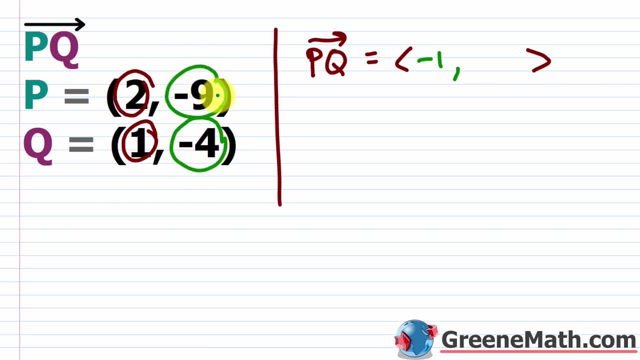 take this one minus this one. Okay, This is from the terminal, This is from the initial. So I want to go: negative four minus a negative nine, which is negative four plus nine, which equals five. Okay, So that's where that terminal point of negative one comma five came from. You go back. 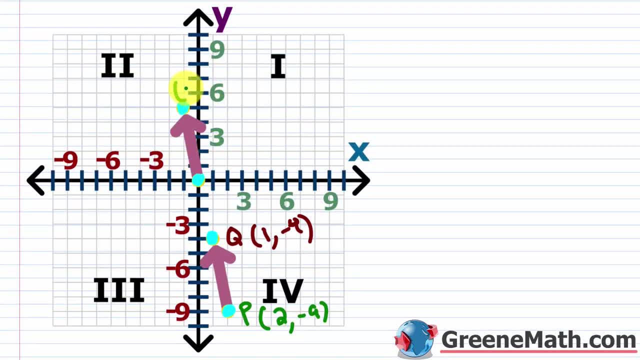 you see, this is one unit to the left and five units up, So this is negative one comma five And you can call this the point Q. Okay, Now the point P is at the origin. Okay, And because of this, a lot of books again. we'll just rename this as the vector V or U or whatever they want. 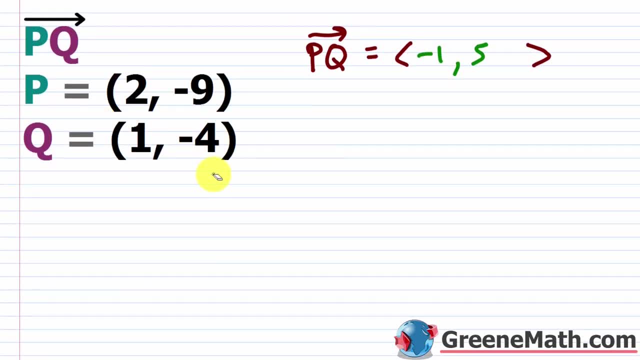 to do? I'm just going to keep it like this. Now, if you want to find the magnitude- okay, and make a little border here- of this vector PQ, Okay. What I'm going to do is just take the square, this first guy, negative one squared, plus the second guy, five being squared, Okay. So the 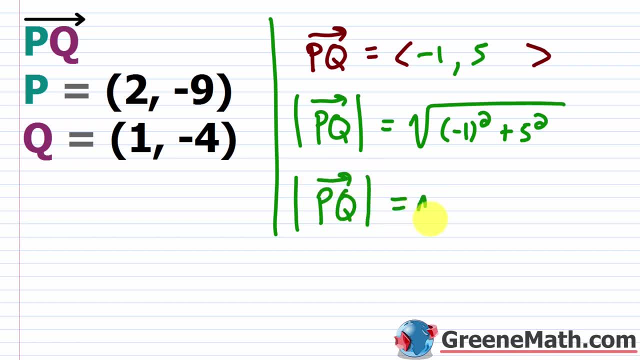 magnitude of PQ. okay, like, this is going to be the square root of negative. one squared is one plus five squared is 25.. So this can be 26.. So it's just a square root of 26.. Now, if you wanted, 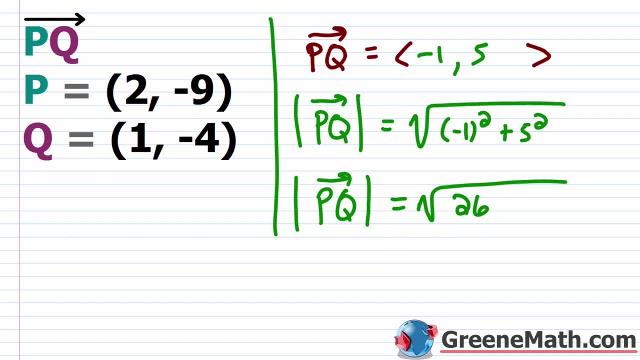 to come over here and use these points again. you could plug into the traditional distance formula. You could say: and I'm just going to label this as the magnitude of this PQ guy, Okay, I'll show you. it's the same. Basically, you're going to subtract this guy minus this guy, So X. 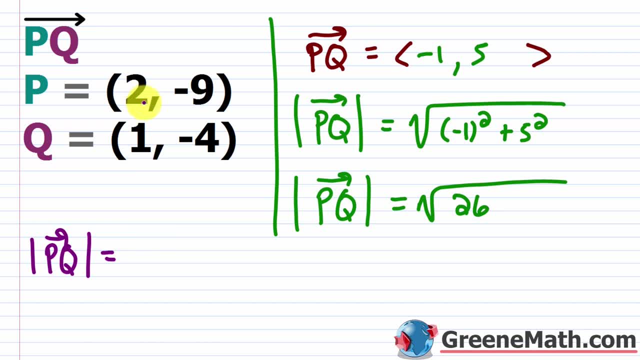 X of two minus X of one, So it's going to be one minus two. Let me, let me write this out: So one minus two, this is squared, Then plus, you're going to do this guy that minus this guy So negative. 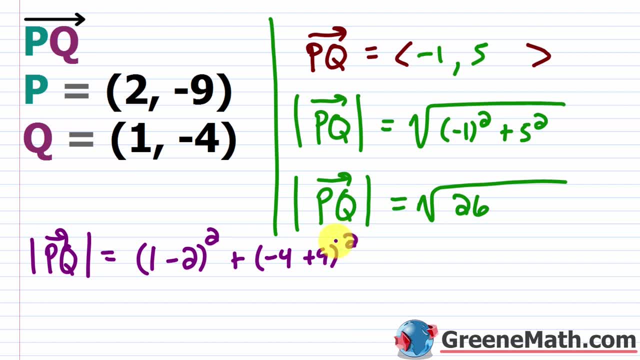 four minus a negative nine is plus nine. Okay, This is going to be squared, and we want the square root of this guy, Okay. So notice that we already did this to find these guys right here. Okay, So we're a step ahead, right? So that's why we do this first and then we don't have to do all this. 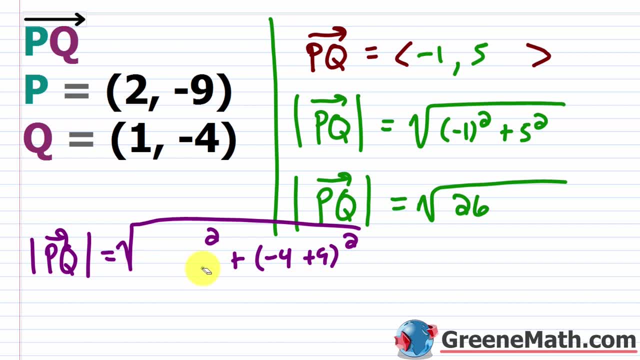 Okay, So one minus two is going to be negative one, So it's negative one squared, which you know. plus nine is five, five squared is 25.. So this becomes square root of 26.. Okay, Just like it is over here. Okay, So you see, it's the same magnitude in each case. Now let's talk a little bit about. 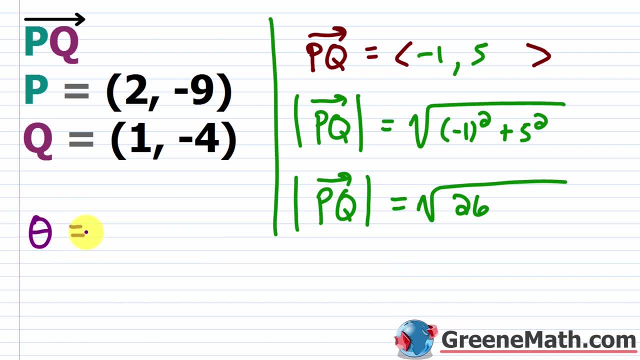 the direction angle. So theta, this is what? well, again, let me actually erase this. Let me just say that the inverse tangent- I think we can kind of skip ahead a bit- The inverse tangent of what? Well, I'm going to take the vertical component, which is five over the horizontal component. 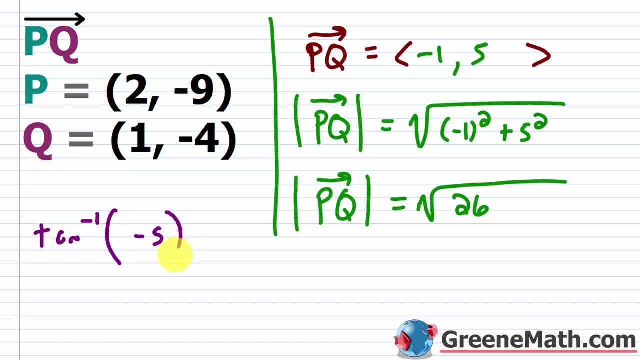 which is negative, one which really I could just write as negative. five Okay, Like this: Now, when you talk about putting a negative as the argument for this inverse tangent function, you're going to get something in quadrant four Okay. So, in this particular case, if we think, 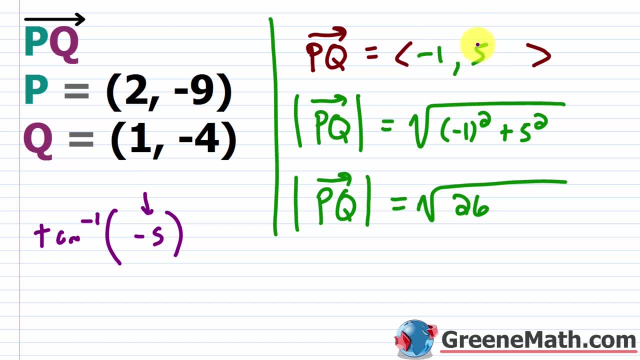 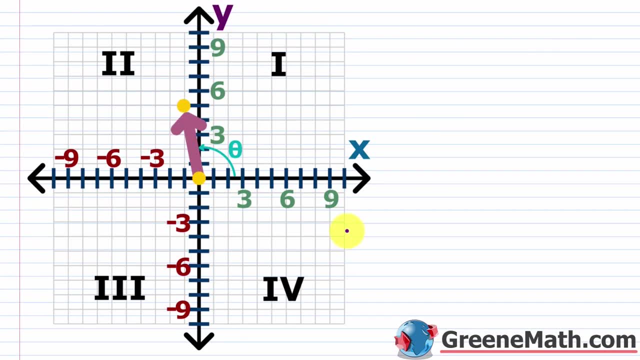 about this. this horizontal component is negative, This vertical component is positive. If I think about it, where am I going to be? I'm going to the left and I'm going up, So I'm going to be in quadrant two. If you want to see this graph on its own, you'll see again my terminal point here. 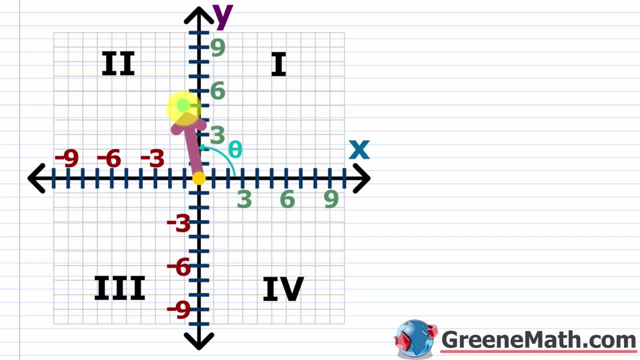 is that we go one unit to the left and we go five units up and you'll see I'm in quadrant two here. So basically, when I do my inverse tangent function, I'm going to end up with something in quadrant four And also I'm going to be rotating clockwise. Okay. So I want to just 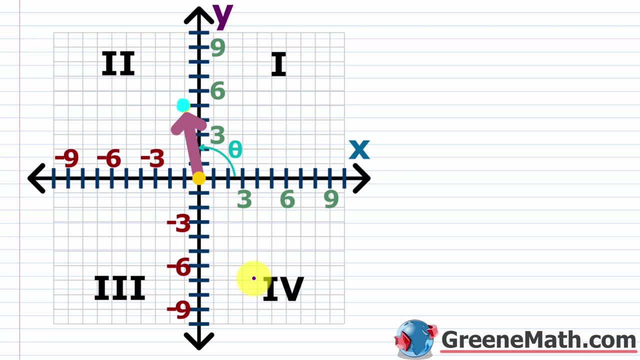 take the absolute value of that and think about that as my reference angle, And then what I want to do in this particular case. I would think about the fact that, okay, if I had an angle of 180 degrees, I want to subtract off and go back by the amount of the reference angle, right? So I want? 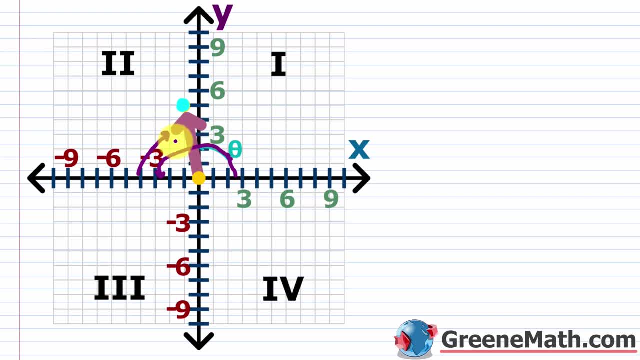 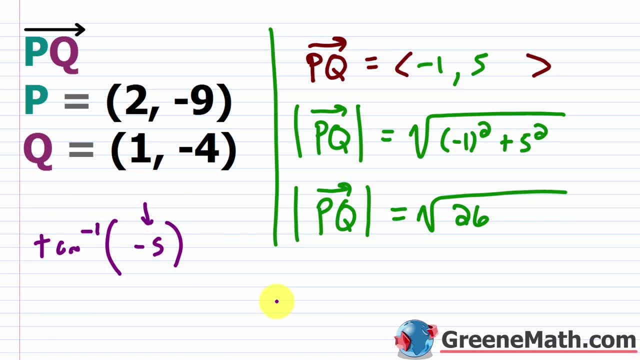 going to get about negative 78 point. let's say six nine. So let me kind of slide this down because I don't think it's going to fit. So we'll put it's approximately negative 78.69 degrees. Now again, what I want to do is I want to think about this in terms of absolute value, So in quadrant. 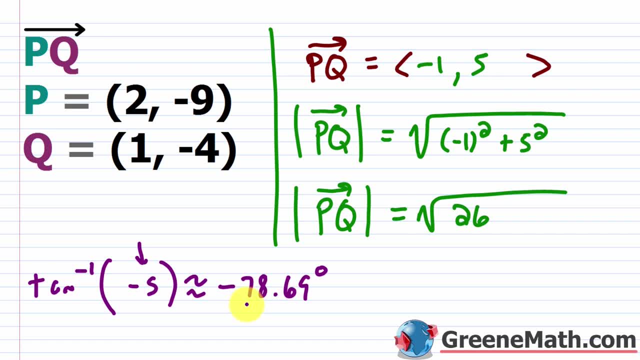 two, I want an angle with a reference angle of 78.69 degrees. So all I'm going to do, get rid of the negative sign. I'm going to say theta is approximately 180 degrees minus this 78.69 degrees And that's going to be about 101.31 degrees. So let's just erase this and put it's. 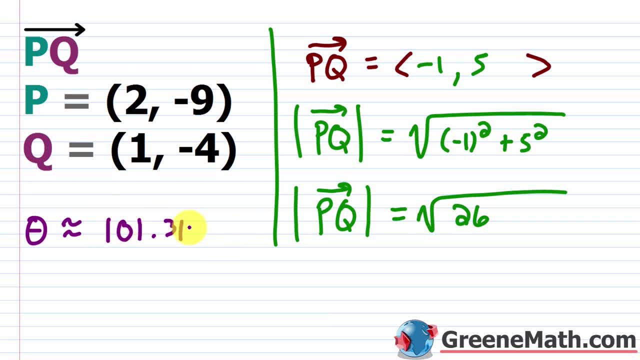 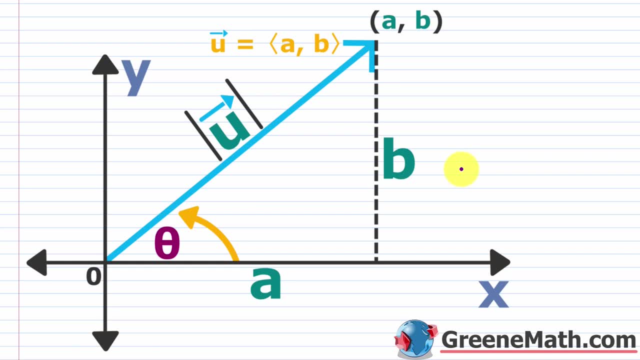 about, or approximately, 101.31 degrees. All right, for the last two examples, we're basically going to reverse things. So now we're going to be given the magnitude of the given vector And we're also going to be given the direction angle, and we have to come up with the component form. Okay, 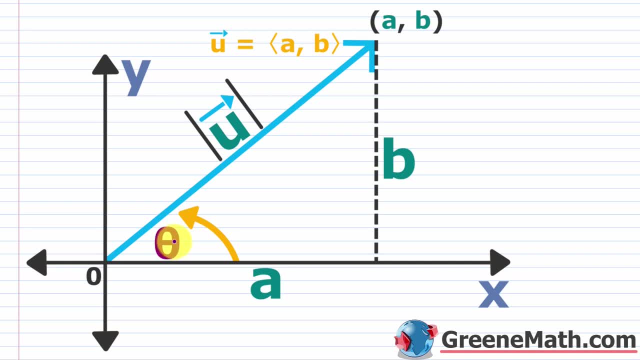 So let's think a little bit about this angle theta And let's think about if I had this guy B and I had this guy A. let's think about some relationships here. I know that the sign of this angle theta is opposite. okay, over the hypotenuse which in 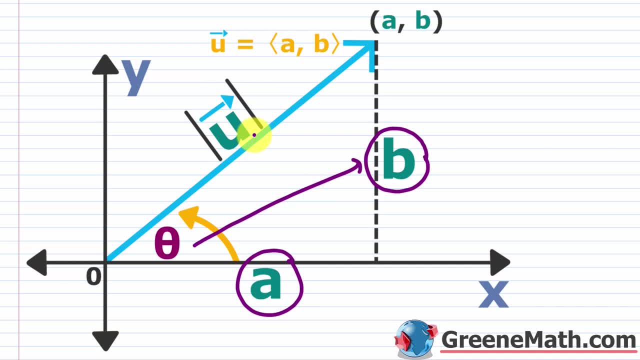 this case would be the magnitude of this vector U. Okay, so I can say that the sign of this angle, theta, is equal to- we'll go ahead and say this- B here, which is the vertical component, over the magnitude of this vector U. 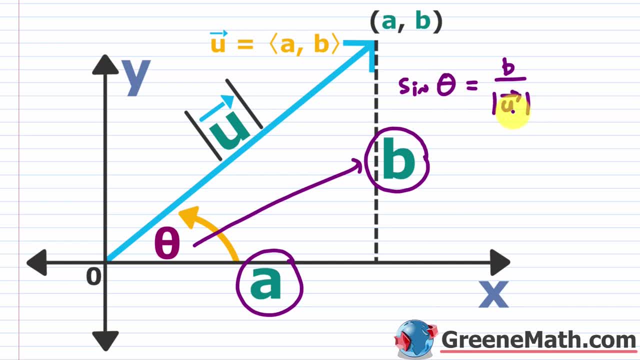 Okay, So I'm going to be given the angle theta and I'm going to be given the magnitude of this vector U, So I should be able to plug in there and figure out what B is. Okay Then also, if I think 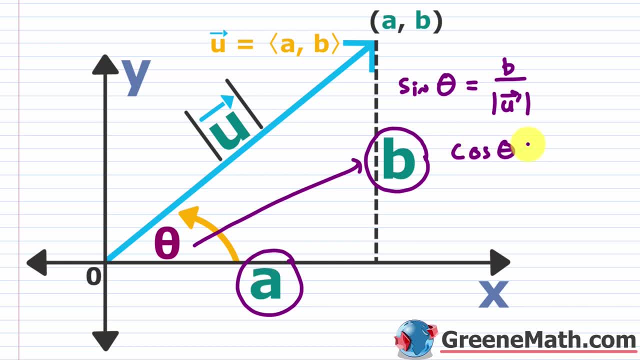 about the cosine. so the cosine of theta, what is that? Well, that's now adjacent, So the- let me erase this- that's the adjacent over the hypotenuse. So this would be A over the magnitude of this U guy. Okay, So we can use these two. we'll just basically solve them for A and B, Okay. 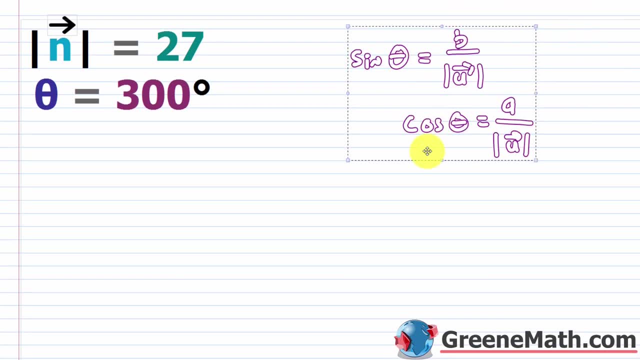 And then we'll plug in and we'll have our answers. So let me just paste this in here and let me drag this over a little bit. We can solve this for A and B. come up with a nice little formula to use here. So basically, if I multiply both sides here by the magnitude of this vector U, you're going. 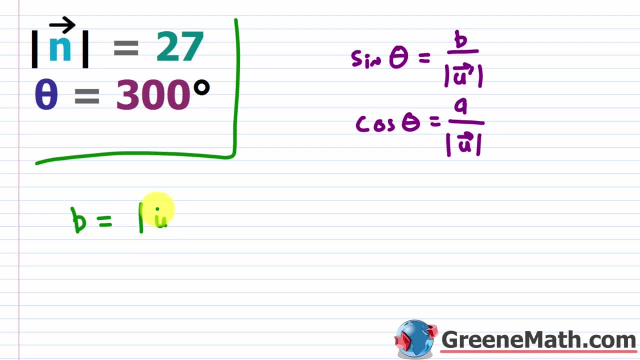 to see that B is equal to, you would have the magnitude of this vector U, and then times the sine of this direction, angle, theta. Okay, Then here, A is equal to the magnitude of this vector, theta. Okay, Let's get rid of this. Now we have a little formula to use, So I'm given the magnitude. 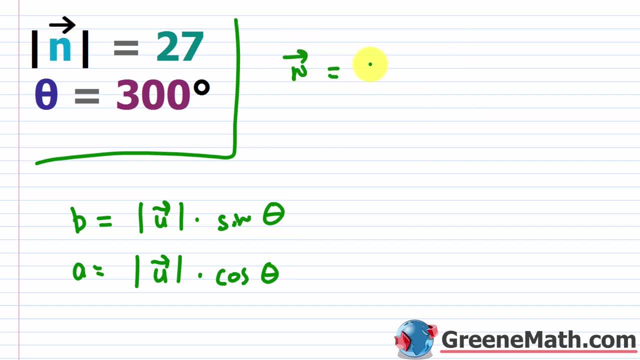 of some vector N, Okay. So I want to find the component form And basically all I'm going to do is think about this and this. So I want the A and the B. So the A goes here, the B goes here, Okay. 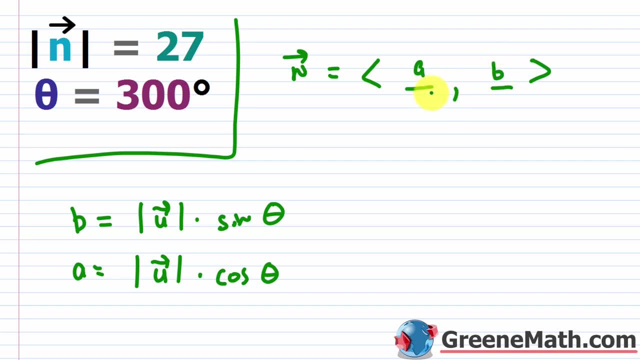 That's all we're doing. So the first one for the A you're going to think about going down here. the magnitude in this case of our vector N is 27.. So I'm going to have 27,. let's put: A equals this. 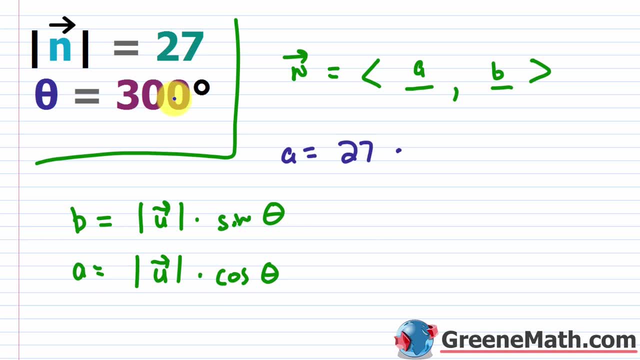 The cosine of the direction angle. theta in this case is 300 degrees. Now, first off, a 300 degree angle is in quadrant four. Cosine is positive in quadrants one and four. Okay, So we know that this guy's going to be positive. Now, 300 degrees has a reference angle of 60 degrees and cosine of 60. 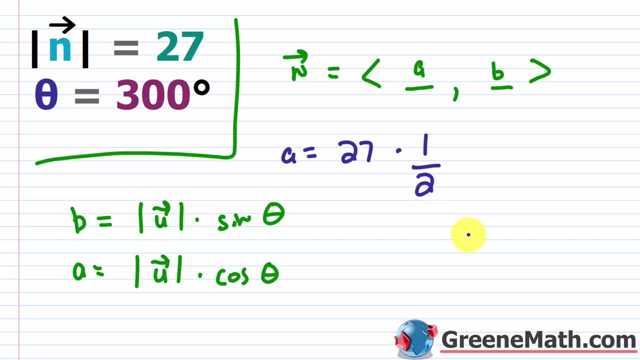 degrees is going to be a half, So I can just put times a half here, and this is basically 27 over two. Okay, So 27 over two. Okay, Then for B. for B, it's equal to what. So in this case again, the magnitude of this vector N is 27. 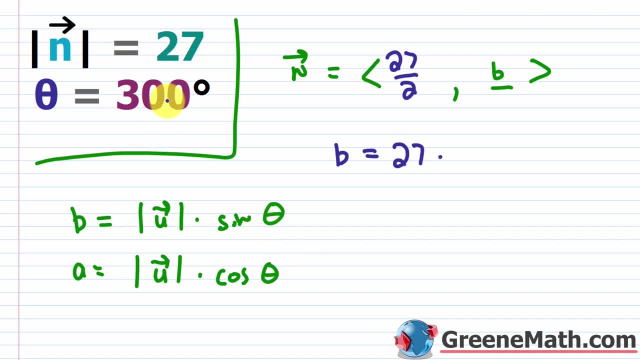 and times the sine of this guy 300 degrees. So again, think about the fact that in quadrant four your sine is going to be negative. right, Sine is positive in quadrants one and two only, So in quadrant four it's going to be negative. Okay, So I'm going to put negative And then the 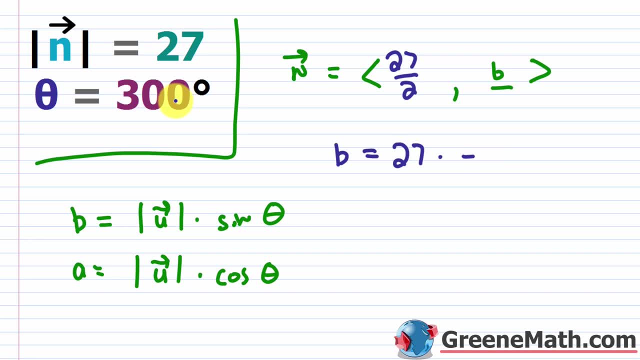 reference angle is 60 degrees. So sine of 60 degrees is square root of three, square root of three over two. Okay, So all this is. you're not going to be able to really simplify this too much. You're going to. 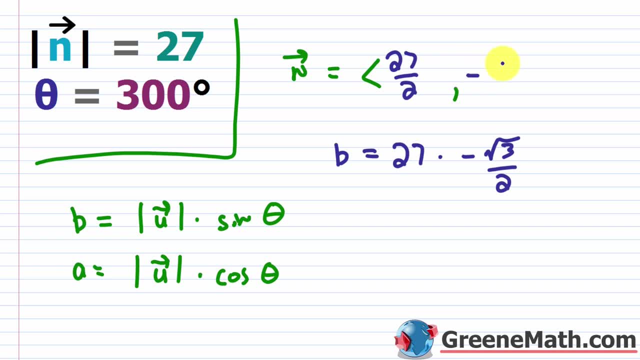 say this is negative. Let me put this out in front. So the negative of 27 times the square root of three over two. Let me close my brackets down. So this would be your component form for this vector N. Let's look at one more of these. So, again, all I'm going to do here. let's go ahead. 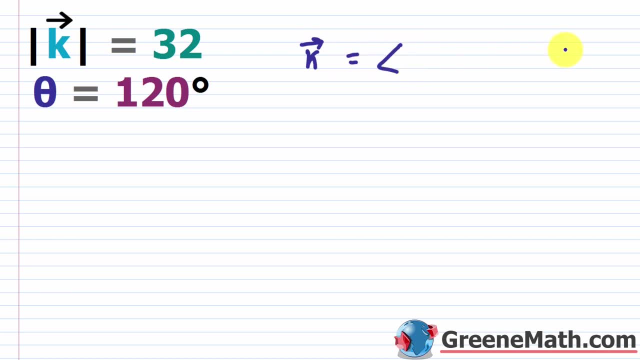 and write this vector K like this is equal to: I'm going to set up my brackets And again, this is A, comma, B. So A is equal to. again with the horizontal, let's see B over two. Okay, So kind of like verifying whether or not these are. 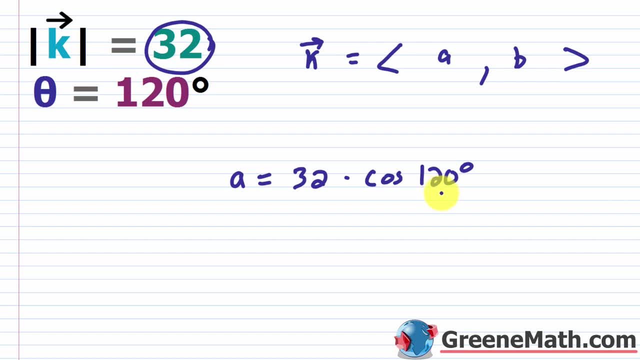 connected, Because you don't want this vector to call out any less than that and say: Putting put in there, cause that's kind of my nuc-. Okay, think about this vector, if we let it call out any less than three over two equals one. 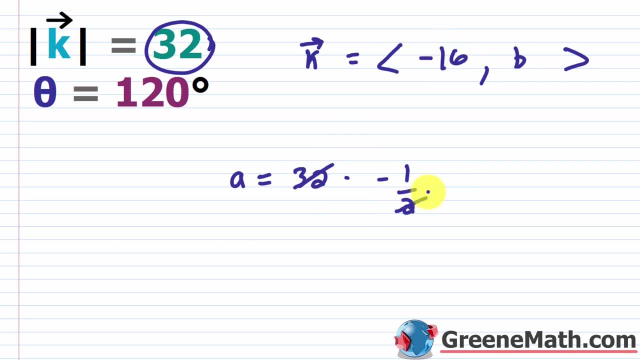 that fits together. Okay ____, Okay, Otherwise I'll just call this vector X ____. So negotiv God. fer rph Sine is negative Right now, So b is equal to. you're going to take the same 32, the magnitude of this vector k times now. 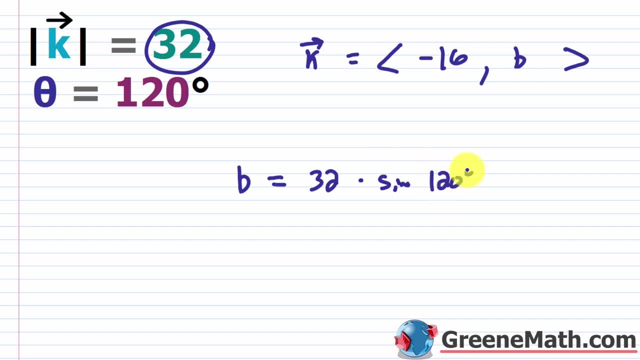 the sine, okay, the sine of this: 120 degrees. While I'm in quadrant 2, okay, I have that same 60 degree reference angle, but now sine is positive, okay. So this is going to be times square root of 3 over 2, and so this is going to cancel with this and give me 16.. So this is 16 times the square. 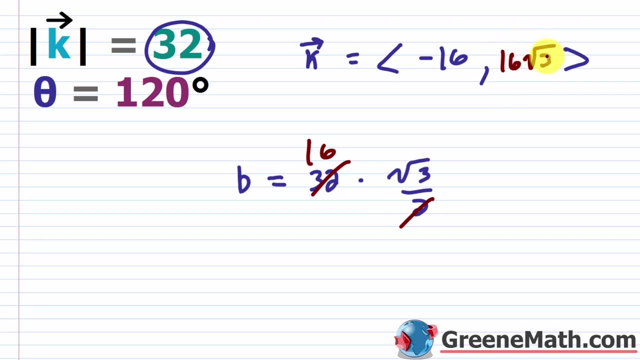 root of 3. okay, So 16 times the square root of 3.. So that's going to be our component form and maybe I should make that 3 a little bit better. okay, For this vector k again, your horizontal component is negative 16. your vertical component is 16 times the square root of 3.. In this lesson, 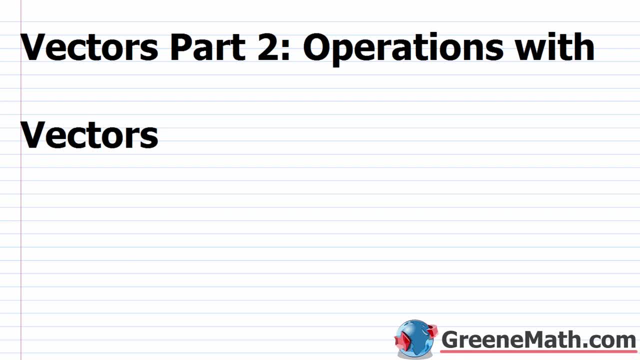 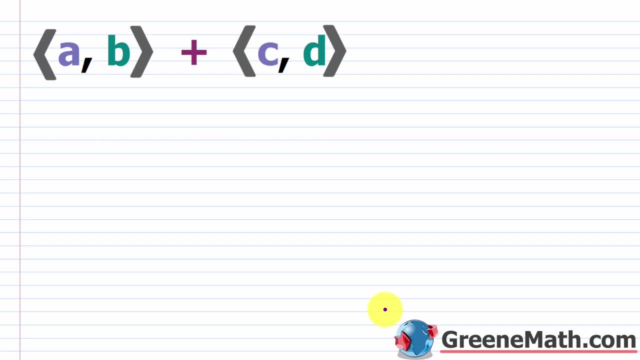 we want to continue to talk about vectors and here specifically, we're going to focus on operations with vectors. All right, so let's start out here by talking about how to add two vectors together. So the sum of two or more vectors is also a vector. This is referred to as the resultant vector, or some people will just call. 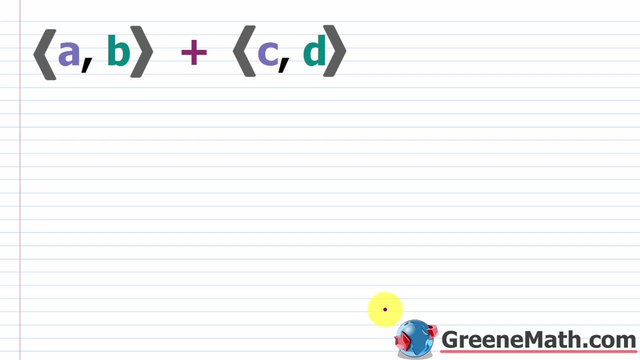 this the resultant. okay, So basically, let's say I have this simple example here, very generic, and on the left I have this vector with a horizontal component of a and a vertical component of b, and I want to add this to this vector on the right, where there's a horizontal component of c. 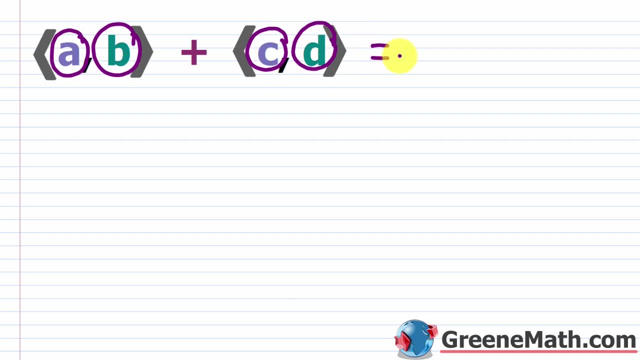 and a vertical component of d. So for my resultant vector, or just the resultant, if you want to say that basically I'm going to do a and b, So I'm going to add this to this vector on the right: a plus c, so a plus c. okay, then I'll do a comma, then I'm going to do b plus d, so b plus d, okay. 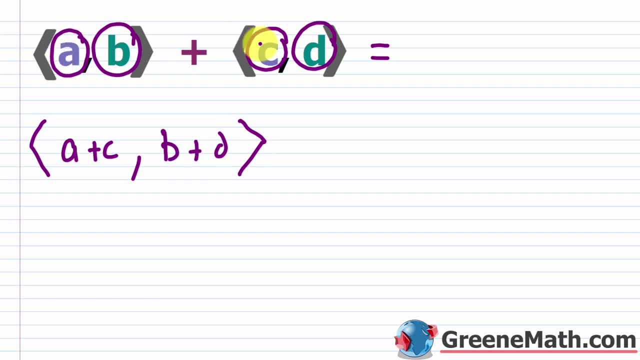 that's all it is. it's very, very simple. You're going to sum these horizontal components so a plus c, that's going to give me the horizontal component for my resultant vector. Then I'm going to sum these vertical components so b plus d, that's going to give me my vertical component. 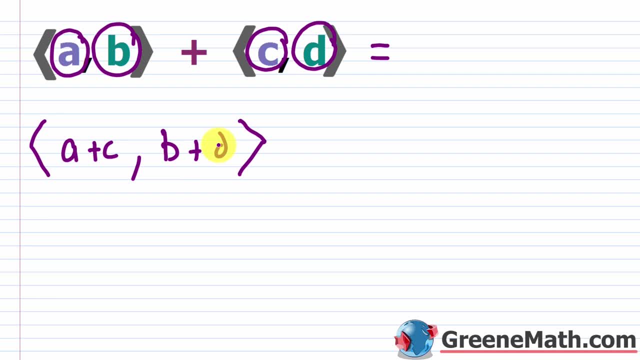 for my resultant vector. and you can do this with more than two. Let's say, for example, I had something like 2 and then 3 here, okay. and then let's say, plus, we'll do maybe 4 and then 5 here. and let's say: 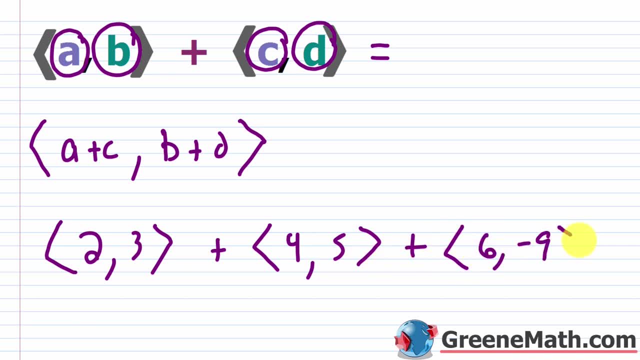 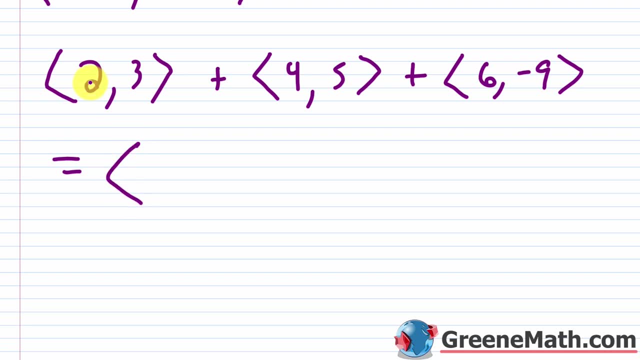 we do plus, let's say we do 6, and then you can even do like negative, so negative, 9.. Okay, so something like this. So all we would do if we wanted to find the sum here, you would say that you would have 2. 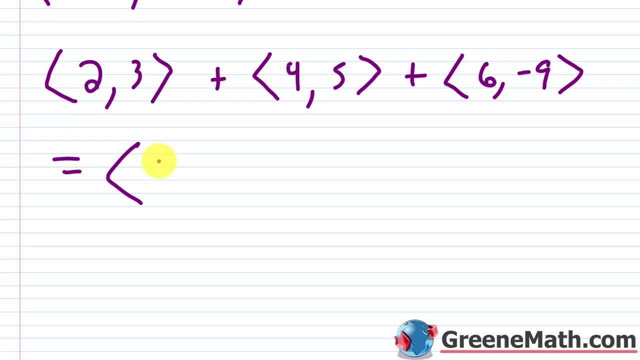 plus 4 plus 6.. So 2 plus 4 is 6.. 6 plus 6 is 12.. Okay, so that's the horizontal component for this resultant vector, and then for the vertical component, you're going to do 3 plus 5 plus. 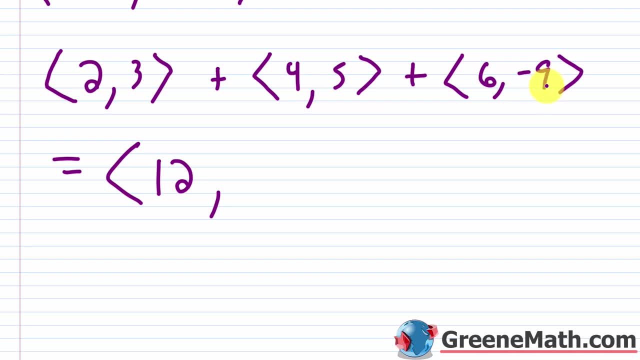 negative 9.. So 3 plus 5 is 8.. 8 plus negative 9 is going to be negative 1.. Okay, so this resultant vector, the horizontal component, is 12 and the vertical component, is negative 1.. All right, let's. 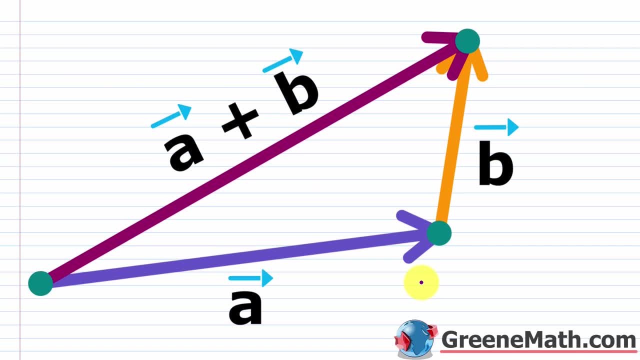 also talk about how to show this geometrically. We can do this with a triangle and we can also do it with a parallelogram. So, using the triangle method, let's think about this: We have this vector a and this vector b. they're being added together. So let's say, I started by just sketching vector a. 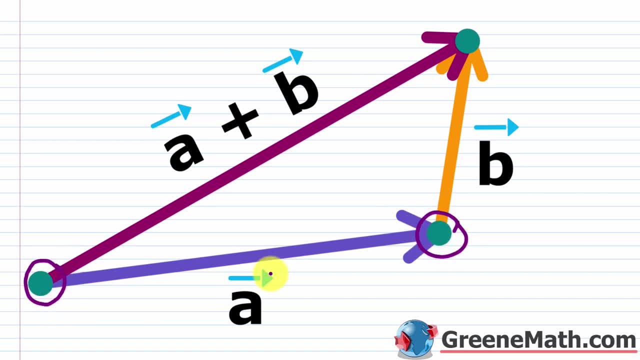 So this is the initial point and this is the terminal point. So I've just sketched vector a. Then for vector b I'm going to use my horizontal and vertical components to sketch this guy. Again, the initial point's here. Your terminal point would be here. let's say Okay, and then your 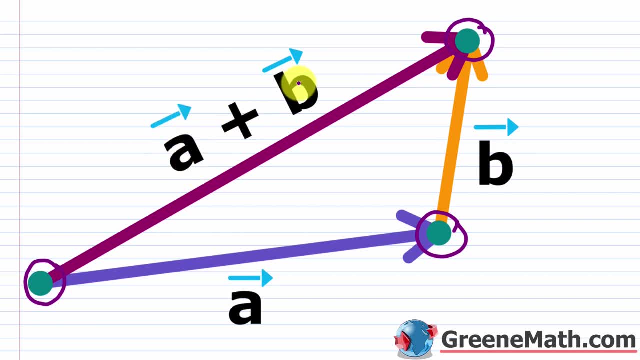 resultant vector, or basically the vector a plus the vector b, is going to be this guy right here, So this vector right here. So you'll notice that the initial point for this vector is going to be the same as the initial point from the vector a. 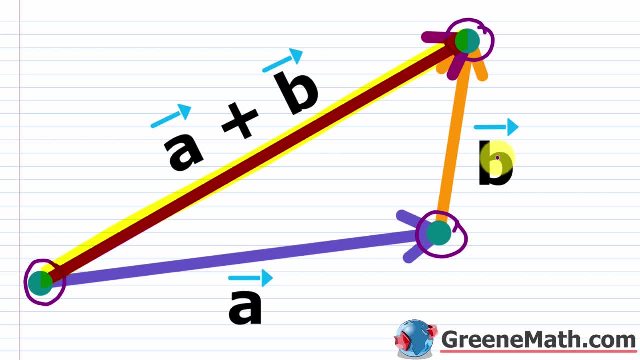 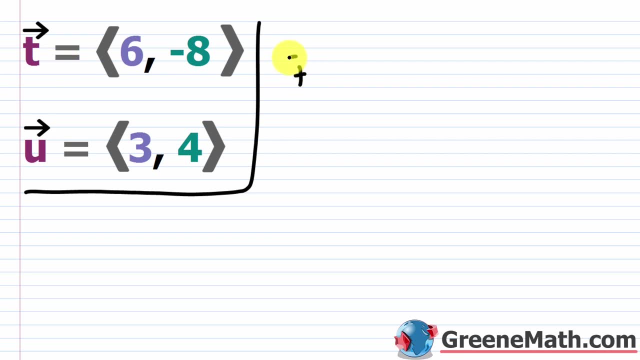 Then the terminal point from this vector is going to be the same as the terminal point from this vector b. Okay, so that's all you're doing. So for this example, let's go ahead and say we have the vector t. Okay, we're going to add to this our vector u, Our vector u. So what is this going to? 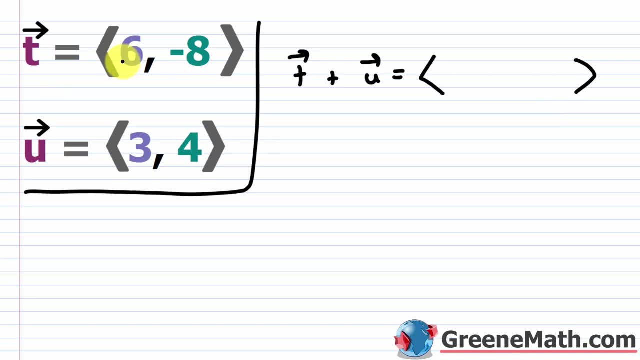 give us. So for the vector t, you have a horizontal component of 6 and a vertical component of negative 8.. For the vector u, you have a horizontal component of 3 and a vertical component of 4.. For the horizontal component, I'm going to take this 6 and add it to this 3.. Right, so just sum the. 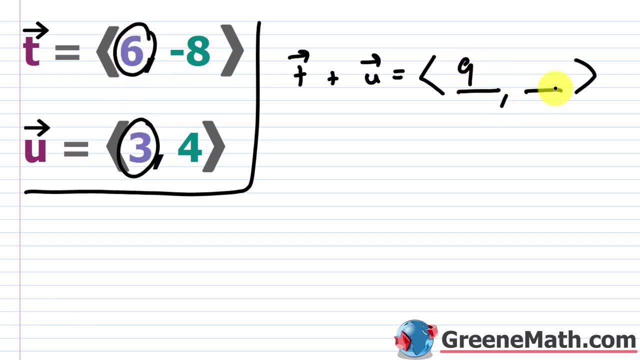 horizontal components. So 6 plus 3 is 9.. Okay, for the vertical component, I'm basically going to sum the vertical components here. So negative 8 plus 4 is going to be negative 4.. Okay, so this guy basically would have an initial point at the origin. Okay, it would have a terminal point at. 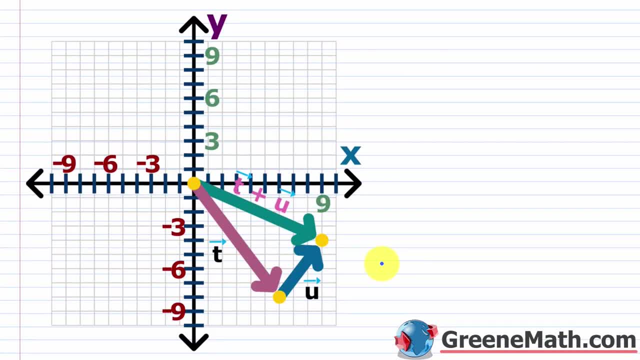 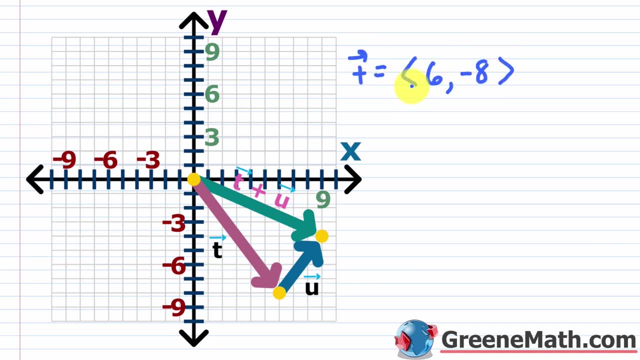 9 comma negative 4.. So let's look at this graphically. Let's start out by just redefining things. So we have this vector t. Okay, in component form this was 6 comma negative 8.. So we had a horizontal component of 6, a vertical component of negative 8.. 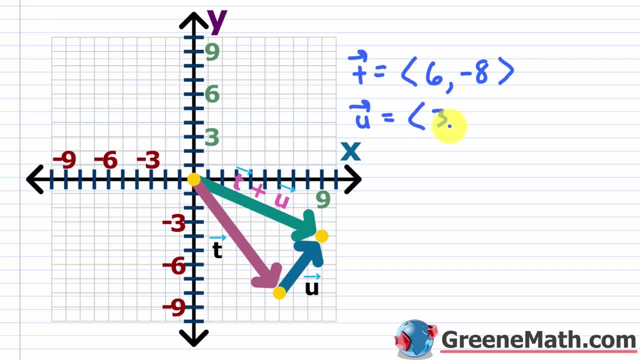 Then for the vector u, we had a horizontal component of 3 and a vertical component of 4.. Then for this resultant vector, so the vector t plus the vector u, we basically what we said 6 plus 3 was 9.. We said: negative, 8 plus 4 is negative, 4.. Right, so a horizontal component of 9 and a. 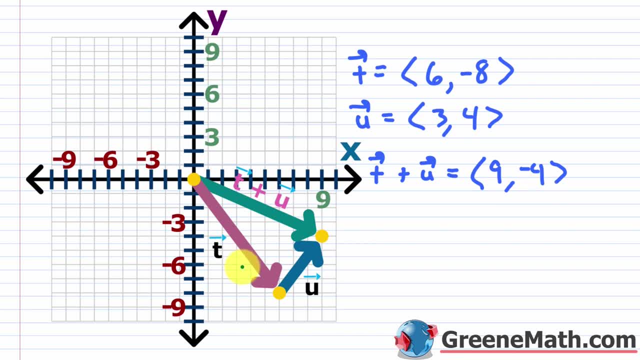 vertical component of negative 4.. Okay so, looking at the graph here, you see, for vector t we started with an initial point here at the origin Right. it's just in standard position, So the terminal point is going to be right here, which is at 6 comma negative 8.. Okay so we want 6 units to the 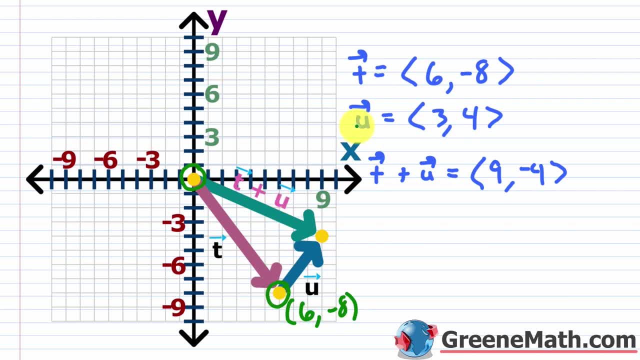 right, and we want 8 units down. So that's, as expected, This vector u. when you try to sketch that now, the initial point has to be at 6 comma negative 8.. So you're using the 3 as the horizontal movement, Right. so I'm just going 3 units to the right and then I'm using the 4 as a vertical. 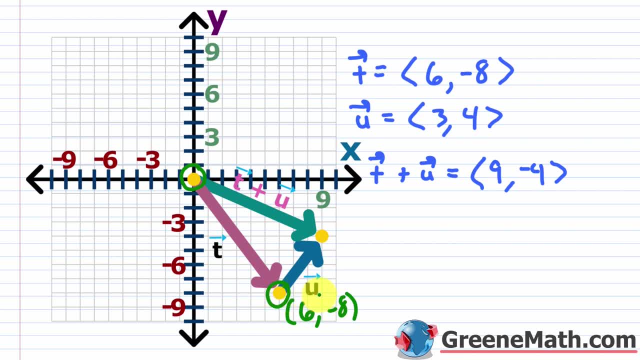 movement. So now I'm going 4 units up, So 1,, 2,, 3 units to the right. that puts me at 9 on the axis. So I'm going to use the 3 as a vertical movement. So I'm going to use the 3 as a vertical. 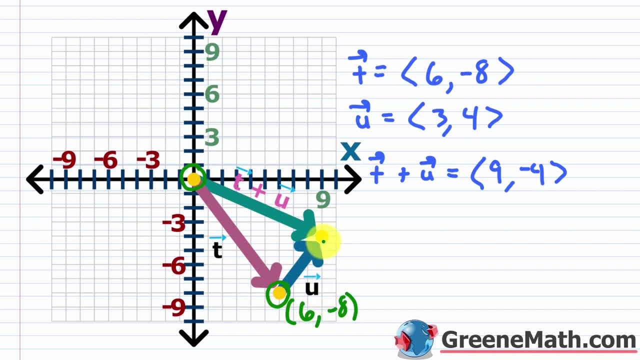 movement. So I'm going to use 3 as a horizontal movement. So this is church. these are 4 units up: 1, 2, 3, 4. that puts me at negative 4 on the y axis. So this point right here would be 9 comma. 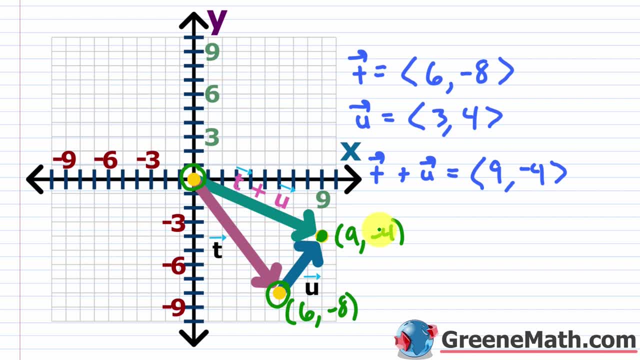 negative 4.. Okay, and this is consistent with what we said, Right? so basically, this vector- right here, this resultant vector, has the same initial point- Okay- as this vector t and has the same terminal point as this vector u. All, right now let's think a little bit about this parallelogram method. 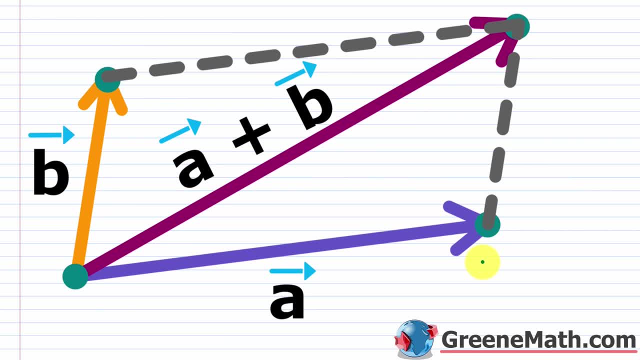 This one's a little bit harder to draw, especially if you're not working on a coordinate plane. but essentially, what you want to do here is have the initial point for the vector a and for the vector b to be the same. okay, so everything's going to have the same initial point. then you'd have 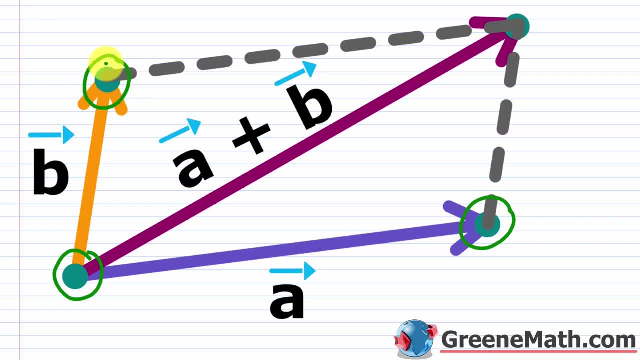 your normal terminal point, your normal terminal point. so these are easy to draw, especially if we're on the coordinate plane. the next part is a little bit more challenging. you're going to complete a parallelogram. essentially, what you're going to do is you're going to take this side. 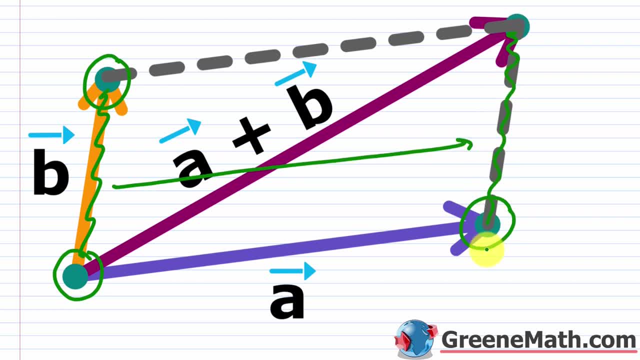 right here and just slide it down. okay, so you would have it like that, okay, and then, basically, this point right here is going to help you set up this diagonal, so this is going to be your resultant vector. okay, now you could also do it this way: okay, where you take this side right here. 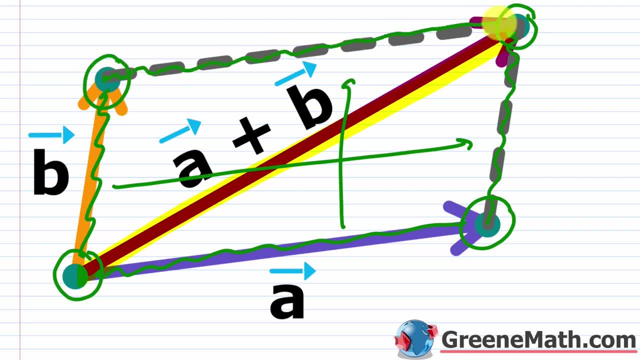 and basically copy it and slide it down, and if you want to form the full parallelogram, you need to do that, right? so, basically, with the parallelogram, okay, in case you're unfamiliar with this, you're going to have opposite sides that are going to be equal in length and they're also 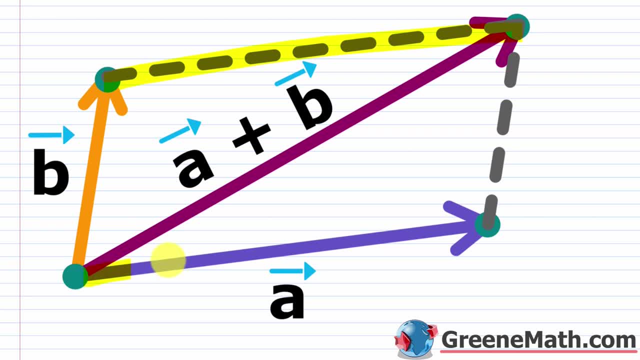 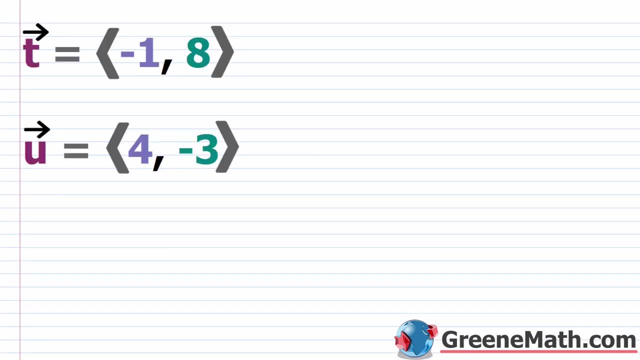 going to be parallel, right. so this side and this side right here are the same length in their parallelograms and they're going to be equal in length and they're going to be parallel, right. and then this side and this side are the same length and they're also parallel. now let's take 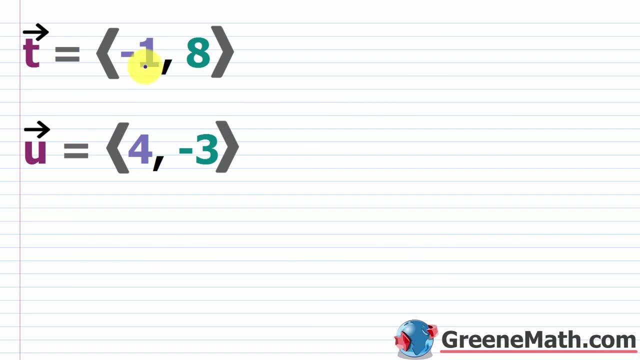 a look at this with an example. we have this vector t, which is a horizontal component of negative one and a vertical component of eight. we have this vector u, which is a horizontal component of four and a vertical component of negative three. so if i did the vector t plus the vector u again, all i 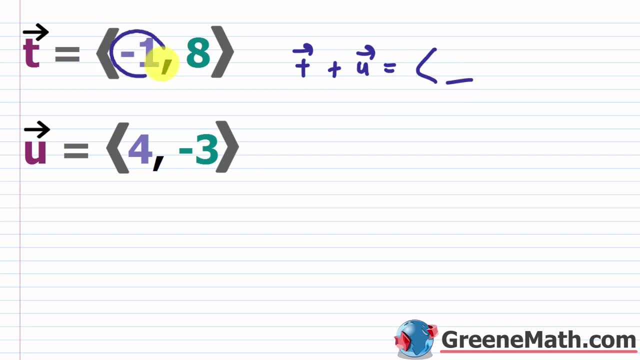 need to do is for this guy right here: for the horizontal component, i'm going to do negative one plus four, so that's just going to give me three, okay. for the vertical component, i'm going to do eight plus negative three, which is going to give me five, okay. so all i want to do is sketch. 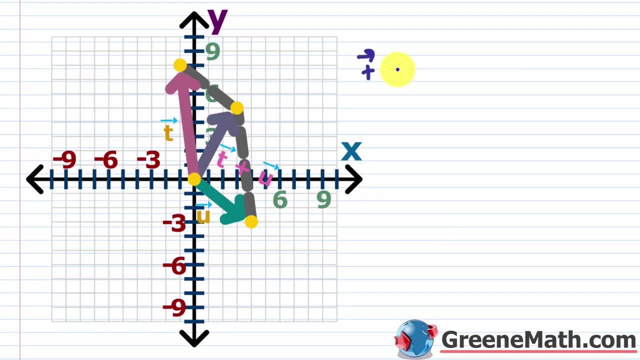 this all right, so let's write this out again. so the vector t is going to be with a horizontal component of negative one and a vertical component of eight. then the vector u is going to have a horizontal component of four and a vertical component of negative three. so the resultant 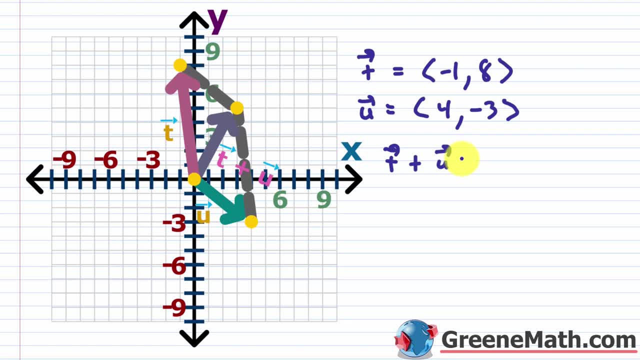 when you do this vector t plus this vector u, this is going to be negative one plus four, which is, and then 8 plus negative 3, which is 5,. okay, So you can see this graphically. It's a little bit more busy than the triangle drawing, but it's still there. So if you look at the first guy, 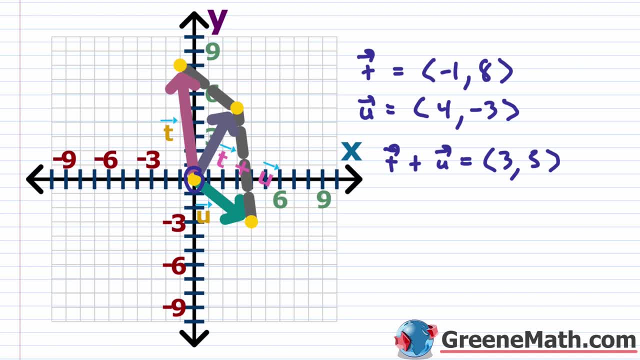 so the vector t- here's the initial point at the origin and then the terminal point right here- is going to be at negative 1 comma 8.. So 1 units to the left, 8 units up. So this is negative 1. 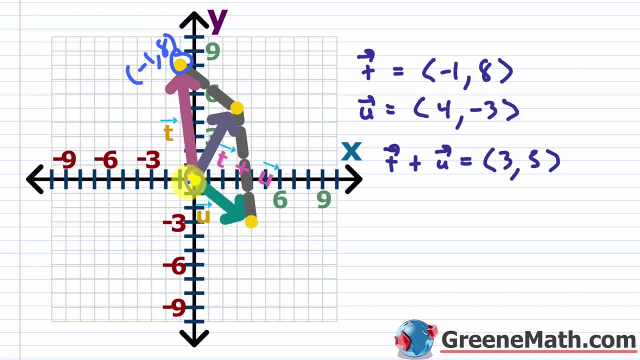 comma 8.. Then if you look at your vector u, okay, your initial point is also at the origin. The terminal point here, okay, would be at this point: 4 comma negative 3, okay, So 4 units to the right. 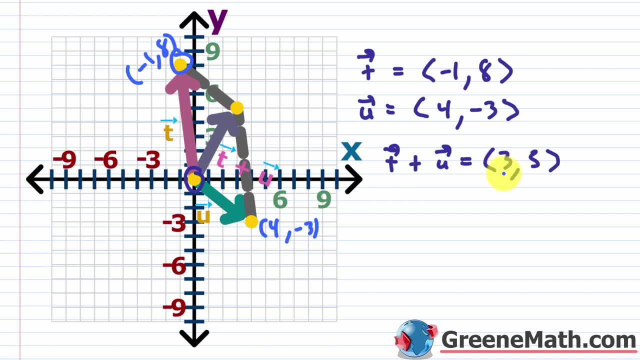 3 units down. And then basically, if you wanted to draw this, you already know the terminal point of this resultant vector is here, okay, which is at 3, comma 5.. And you could basically sketch: this guy right here, okay, and this guy right here, Those sides there again, this side right here. 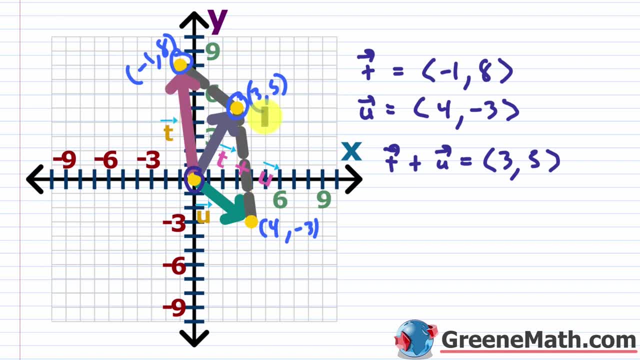 okay, is going to be the same length and parallel to this side right here, Then the other one's the same thing. So this side right here and this side right here- okay, are going to be the same length, right here, same length, and then are also parallel, okay? So when you look at this guy, 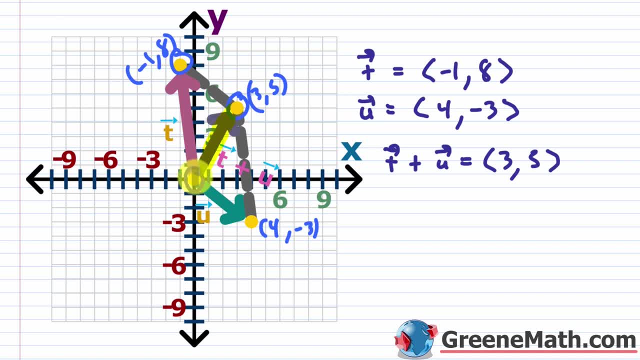 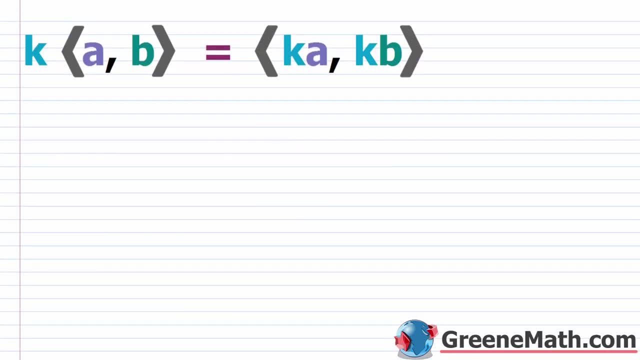 you would then draw this vector here, okay, where basically the initial point is the same as the other two vectors and your terminal point is right there, okay, So it's going to be at that 3 comma 5.. Okay, let's talk about this. multiplying a vector by a scalar- Also very easy. So let's say: 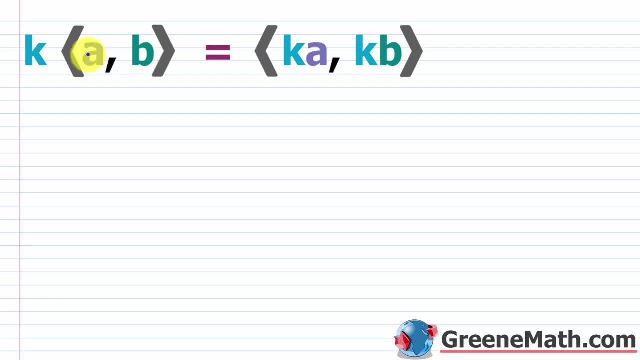 you had some real number, k, and it was multiplied by this vector with a horizontal component of a and a vertical component of b. Well, the result of this is going to be a vector with a horizontal component of k times a and a vertical component of k times b. okay, So the reason they call it a. 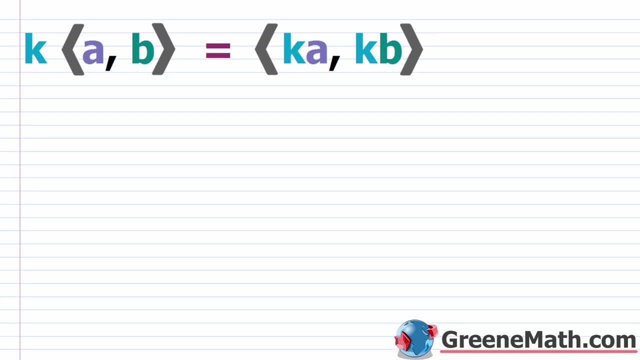 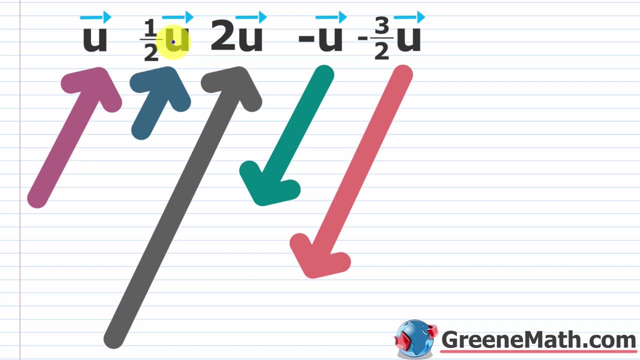 scalar is. you can think about this as scaling your vector. okay, So graphically, you can think about it like this: Let's say we had some vector u. okay, So this is u to start. If you had half times this vector u, we can see that it's half as long. okay, If you had two times this vector u. 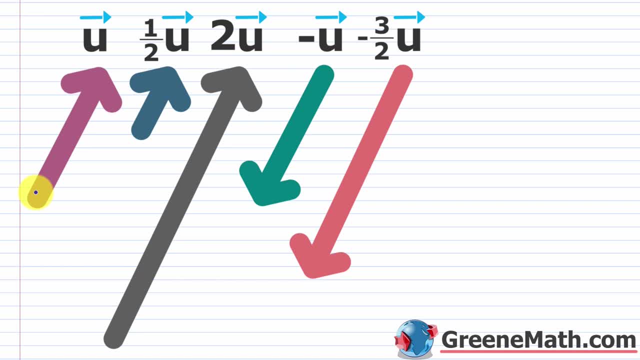 now it's twice as long, okay, compared to this original vector u. Now, when you get a negative involved, what it's going to do is it's going to give you an opposite direction, okay. So, basically, if I had the negative of this vector u, it's going to flip the direction. 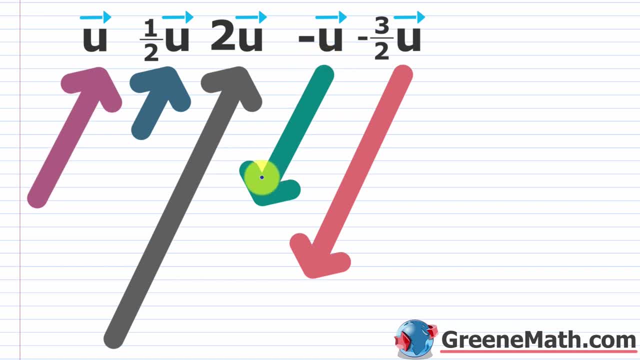 right. So it's the same length, but the direction is flipped right. It's the opposite direction. Then if I had negative three halves times this vector u, well, now it's the opposite direction. basically, compared to this original vector u, in terms of its length, it's going to have one half. 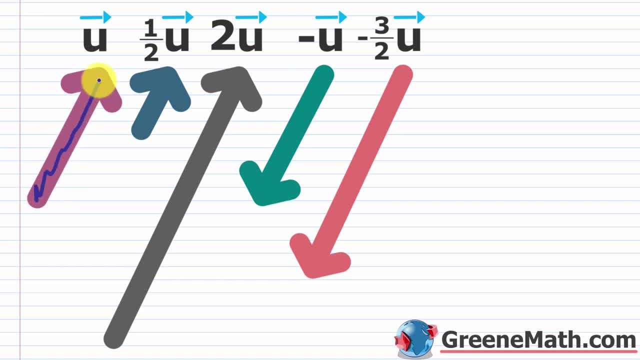 of the vector u added on right. So it's like I took this vector right here and added this vector right here onto it and then I gave it the opposite direction to form this vector here which is negative, three halves times the vector u. okay, Let's find the negative two times the. 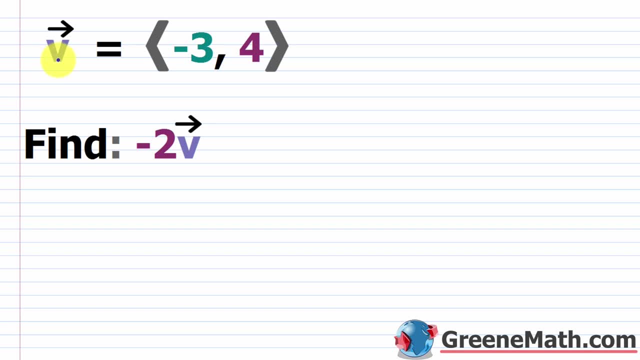 vector v and then I'll show you this graphically. So we have the vector v. horizontal component is negative three, vertical component is four. So if I wanted negative two times this vector v, then all I would do is negative three times negative two, which is positive six. 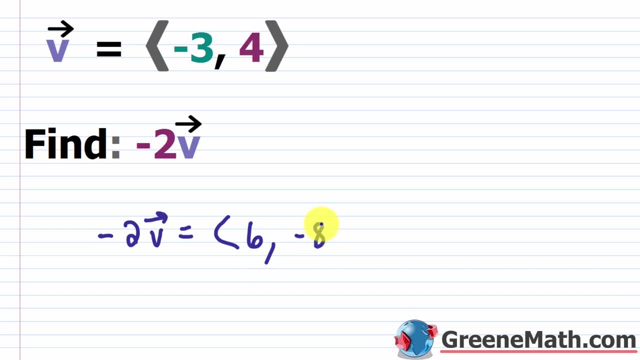 and then I would do negative two times four, which is negative eight. okay, So this guy right here, this negative two times this vector v, is going to be negative three times this vector u, six for the horizontal component and negative eight for the vertical component. Now, graphically, 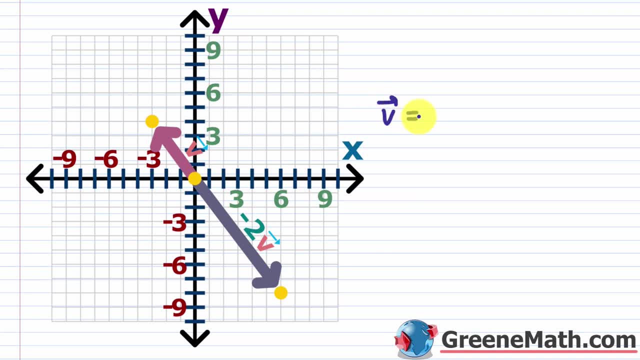 the original vector v- again, when we look at this, is going to have a horizontal component of negative three and a vertical component of four. okay, So you see, it starts at the origin. that's the initial point, and then the terminal point is right here, again at negative three. 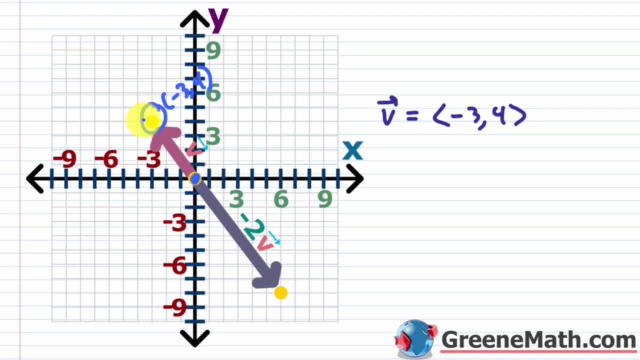 comma four. okay, So three units to the left, four units up. Now, if I look at negative two multiplied by that vector v, so negative two multiplied by this vector v- again I'm scaling because this guy is twice as long. okay, That's the two part, and then it's going in the opposite. 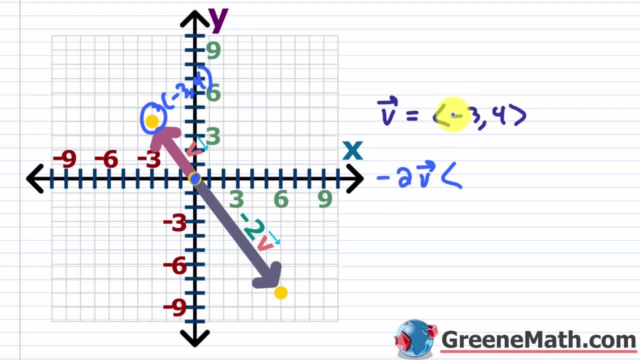 direction. that's the negative part. okay, So basically I'm multiplying everything here by negative two. so this is six and this is negative eight, and you'll see that the initial point is the same. the terminal point is here. I went six units to the right, eight units down. this is six. 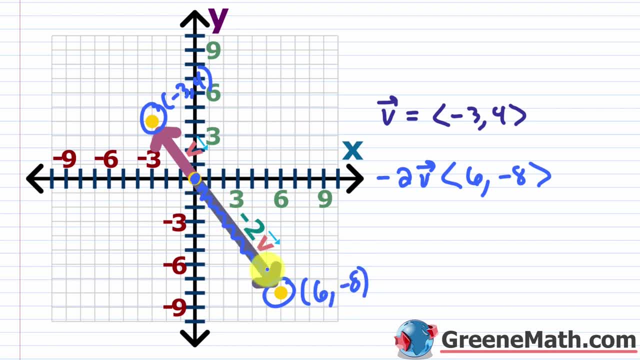 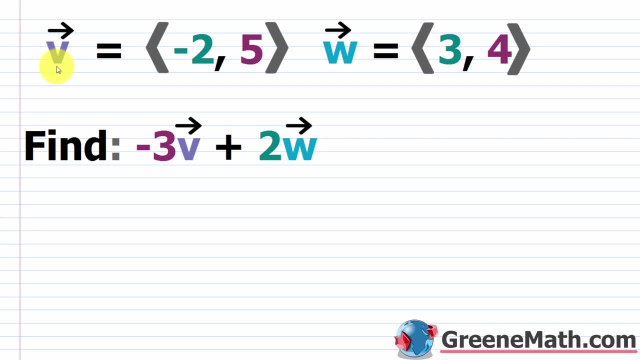 comma negative eight. okay, So you can see, this guy right here is twice as long and it's also going in the opposite direction. Okay, so let's combine these two concepts together. So now we have this vector v, horizontal component of negative two right here, and this vector v. 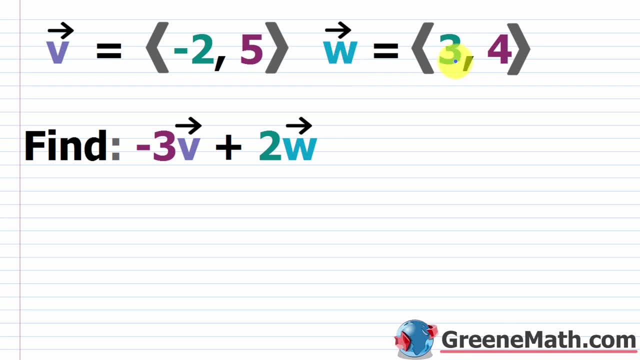 vertical component of five, and then we have this vector w with a horizontal component of three and a vertical component of four. We want to find negative three times the vector v plus two times the vector w. okay, So all I'm going to do is set this up and say negative three times this vector v. 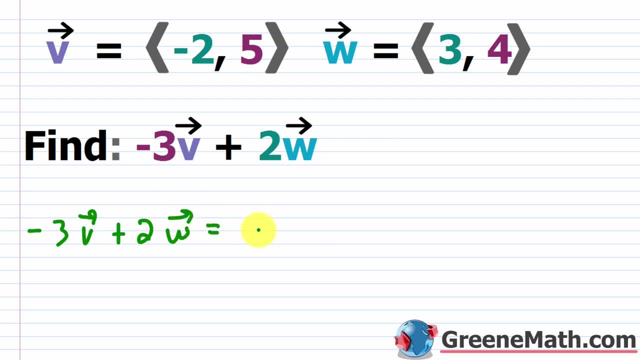 plus two times this vector w is equal to. I'm just going to put a negative three out in front of this, so negative two and then five is inside, and then plus, I'm just going to put a two out in front of this, and then I'm going to put a three and then a four inside. okay, So that's all I'm. 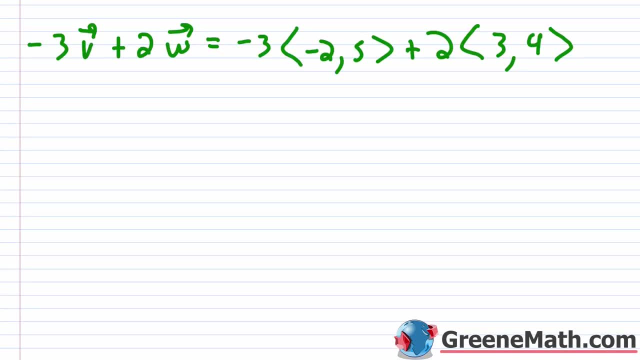 doing So what I'm going to do is just first multiply. So let me copy this down, or I could just put equals. to keep this going, I'll say: basically, each part of this is going to get multiplied by negative three. So this would be negative three times negative two, which is six. 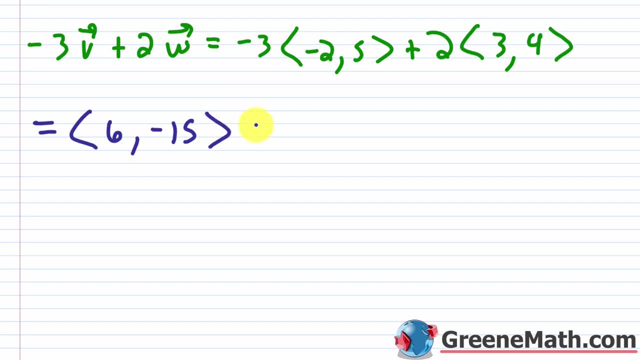 and then negative three times five would be negative 15,. okay, Then plus two times three is six, and then two times four is going to be eight. okay, So now I just want to find the sum. again, very easy, I'm going to add the horizontal components. so six plus six is 12.. Then I'm 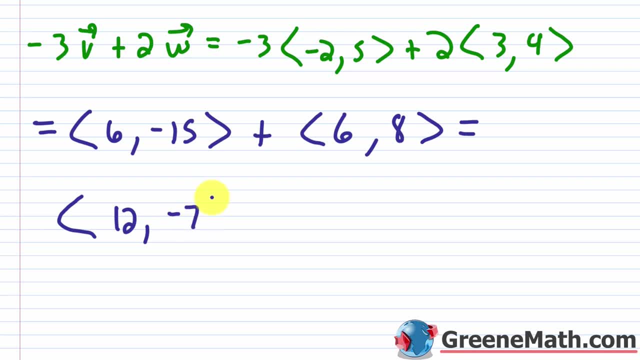 going to add the vertical components. so negative 15 plus eight is negative seven. okay. So in the end, this negative three times this vector v plus this two times this vector w gives me this vector okay, with a horizontal component of 12 and a vertical component of negative seven. All right, 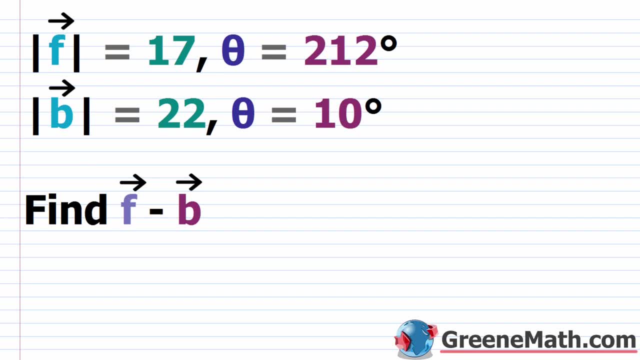 let's wrap up the lesson and look at something that involves a concept from the last lesson. So we have: the magnitude of this vector f is 17,. theta is 212 degrees. The magnitude of this vector b is 22,. and the direction angle: theta. 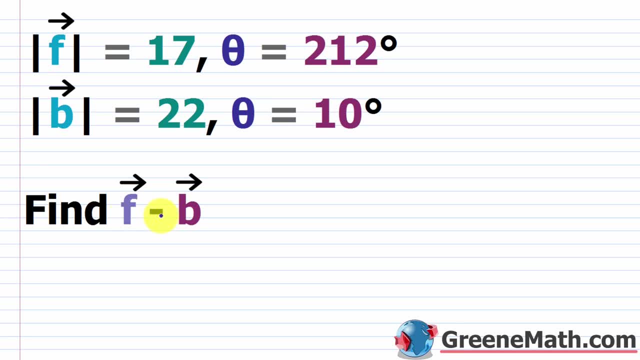 is 10 degrees. So what if I wanted to find the vector f minus the vector b? What would I do? Well, first I need to find the horizontal and vertical components for each. So remember how to do this For the vector f. to set this up, I would do what I would take my magnitude 17,. 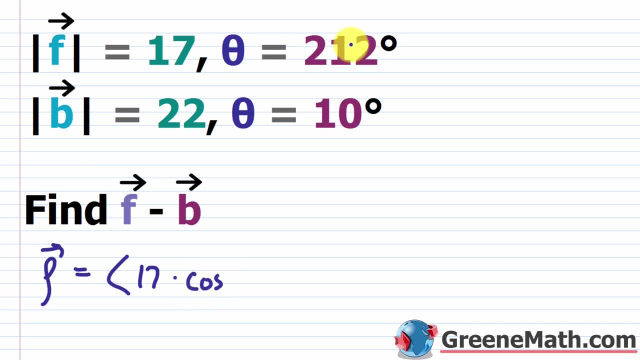 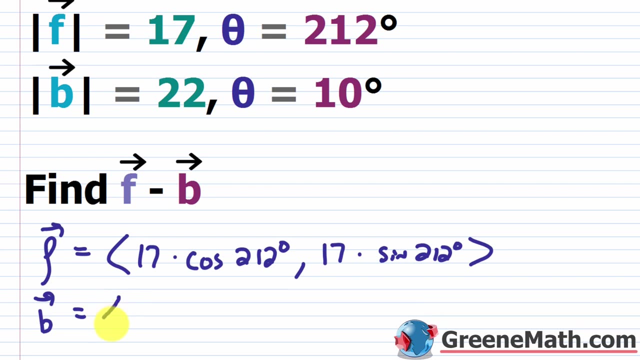 and for the horizontal component, I'm multiplying by the cosine of this direction angle, which is 212 degrees, and then for the other one, it's going to be 17 times the sine of 212 degrees. okay, That's all I'm doing. Then, for b, this vector b, what I would do is I would do 22 now. 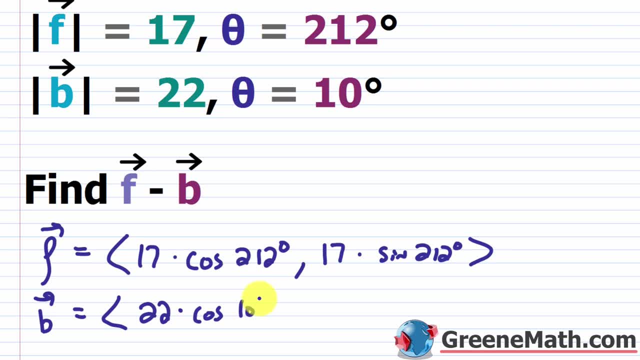 the magnitude of this guy times the cosine of- in this case, 10 degrees, okay. And then I would do 22 times the sine of this- 10 degrees as well, okay. So you can punch that up and get approximations. 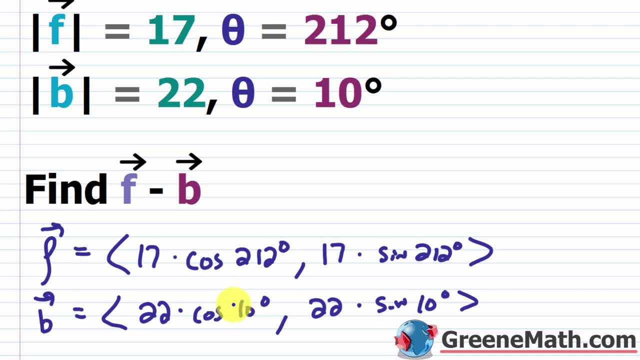 and then set up your subtraction. If you want to, you can go ahead and do this all in one step. So we could basically say: 17 times the cosine of 212 degrees minus 22 times the cosine of 10 degrees. okay, Then comma, you would have. 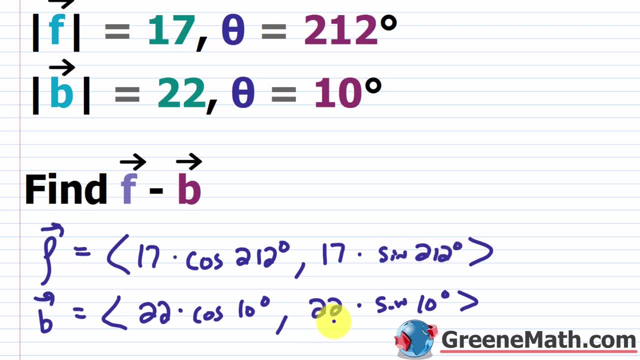 17 times the sine of 212 degrees, minus 22 times the sine of 10 degrees. Up to you. how do you want to do it? You get the same answer either way. Actually, the rounding might be a little bit different, but let's just go ahead and do it the long way. Let's get some practice. So first, 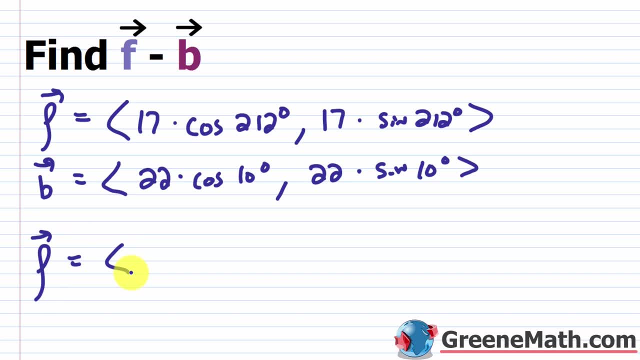 I'm just going to say the vector f is going to be- let me put approximately here, because I'm going to approximate this- 17 times the cosine of 212 degrees. I'll say that's about negative 14, point. let's just go ahead and say 42,. okay, This guy. 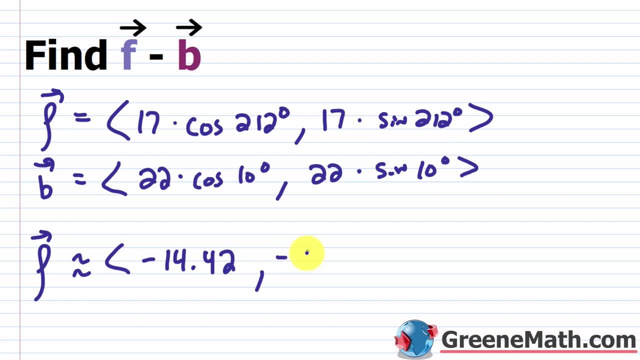 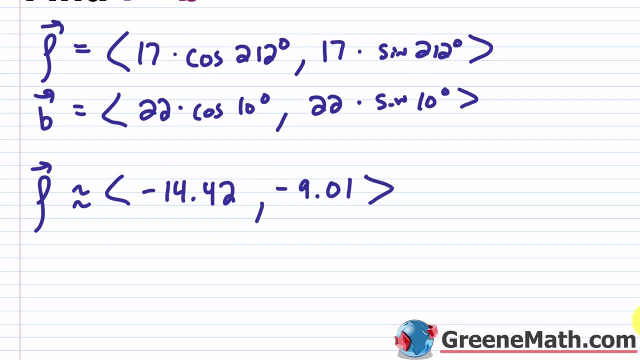 17 times sine of 212 degrees is going to be about negative 9.01,. okay, So this is my vector f And again, this is an approximation. So let's scroll down and get a little bit more room so we can stay. 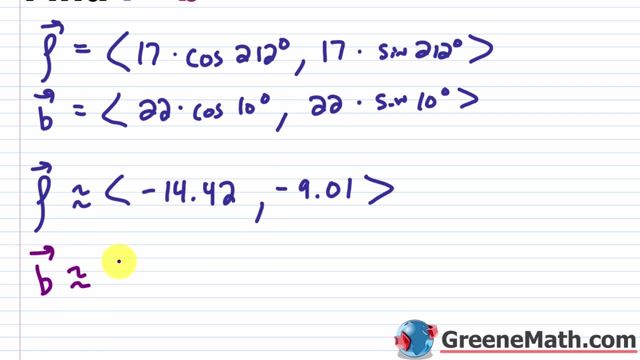 on the screen. I'll do my vector b now. So this is approximately- we'll go ahead and set this up- 22 times cosine of 10 degrees. It's going to be about 21.67,, so 21.67.. And then 22 times the sine. 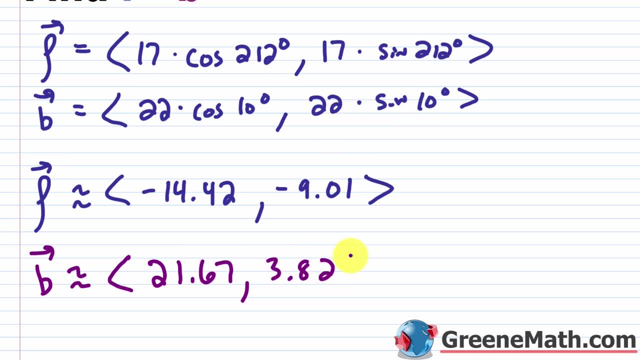 of 10 degrees is going to be about 3.82, okay, So now let me make this a little bit better. And let me change these, make them a little bit better, a little bit better, okay. So now, 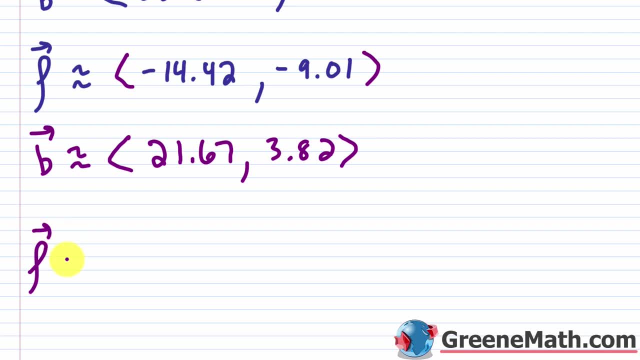 if I come down here, if I want to do the vector f minus the vector b, all this is going to be is minus 21.67, comma. I'm going to have negative 9.01 minus 3.82,. okay, And I put equals, it should. 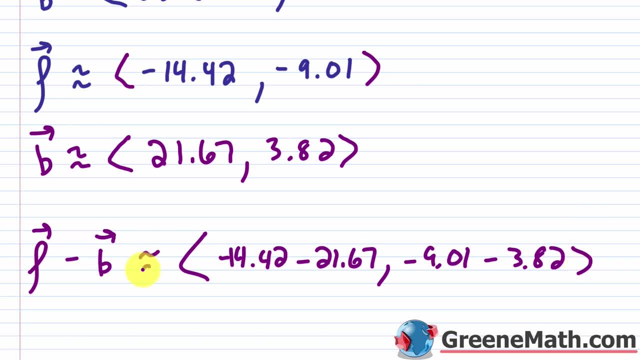 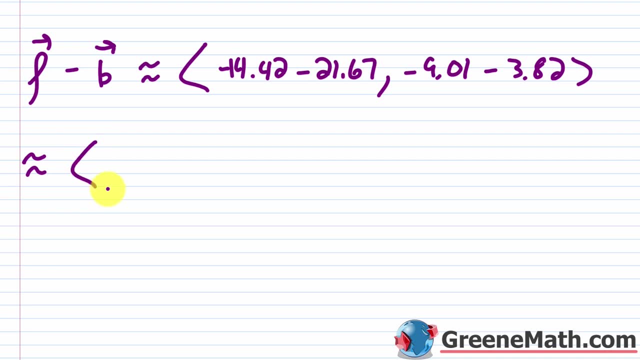 probably be approximately, to be more precise. So let me go ahead and put that like that, okay, to make that better, And let's just go ahead and correct this out. So I'll say this is approximately, and I'll put my little symbol there. say: about negative 36.09, right For negative: 14.42 minus. 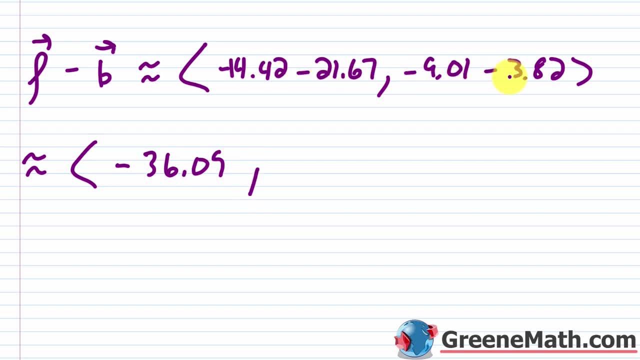 21.67.. Then over here, negative 9.01.. Minus 3.82.. We'll say this is negative 12.83.. Again, this is an approximation. okay, So the vector f minus the vector b, the horizontal component, would be about negative 36.09,. 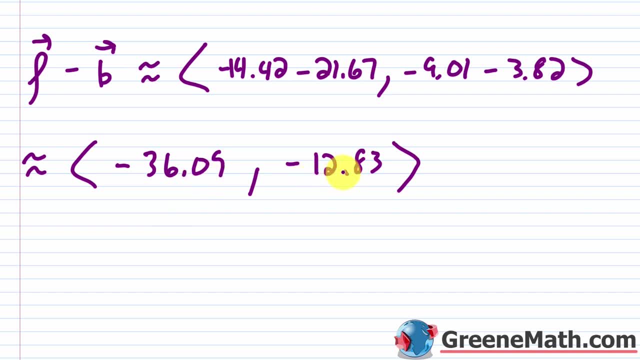 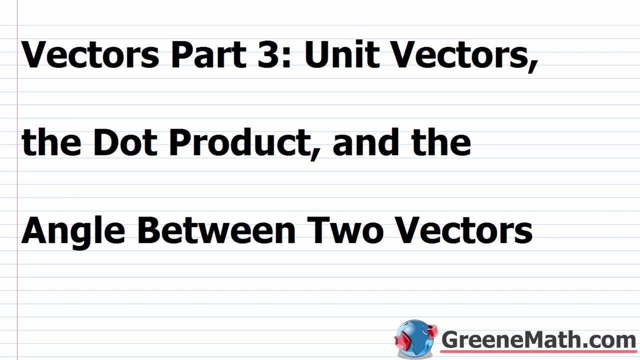 and the vertical component would be about negative 12.83.. In this lesson we want to continue to talk about vectors And here, specifically, we're going to focus on unit vectors, the dot product and then the angle between two vectors. All right, so to start the lesson we're going to talk about, 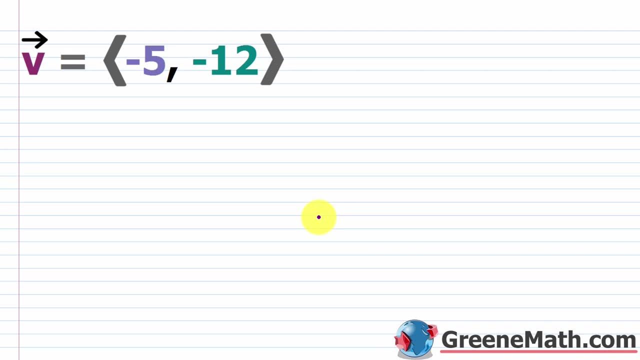 something called a unit vector And we're going to talk about a unit vector and we're going to. So a unit vector is just a vector that has a magnitude of one. okay, So let's say that we denote our unit vector with a? u. okay, When you work with a unit vector, you're going to have a. 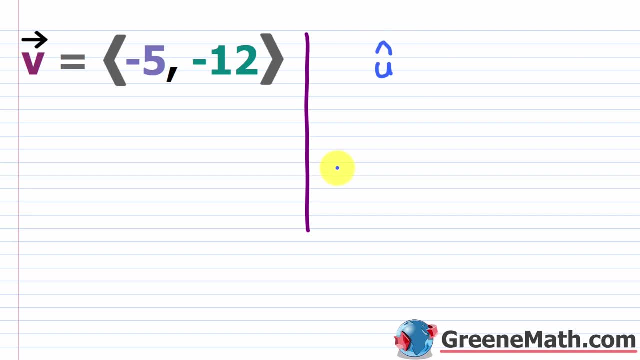 special notation. Some people call this a cap, Some people call it a hat, But basically this tells you you have a unit vector, okay, And if you have a unit vector, the magnitude of this unit vector- again let's call it u- is always going to be equal to one. So for some problems, 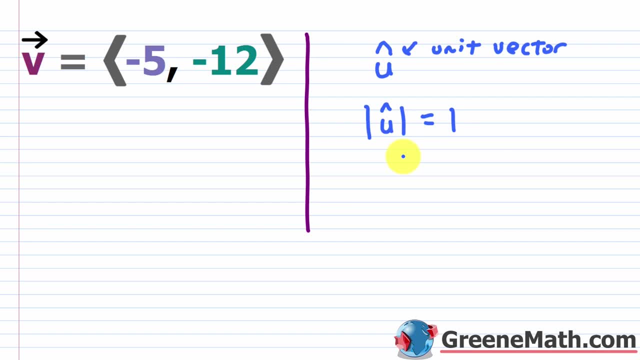 you're going to be asked to find a unit vector- Let's call it u- That has the same direction as a given non-zero vector- let's call it v. And basically, to solve this type of problem, you're just going to take your vector v and divide it by the magnitude of 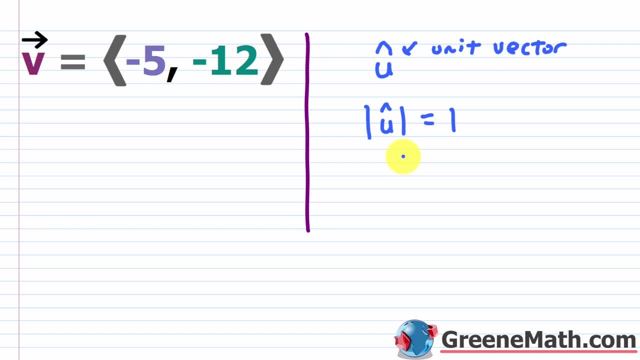 that vector v. okay, And that's going to give you your unit vector u. Now, if you're confused by me saying it, it's okay. The formula is very, very simple. So, basically, this unit vector u is equal to the vector v. okay, So the vector v divided by the magnitude of that vector v. okay, So you can. 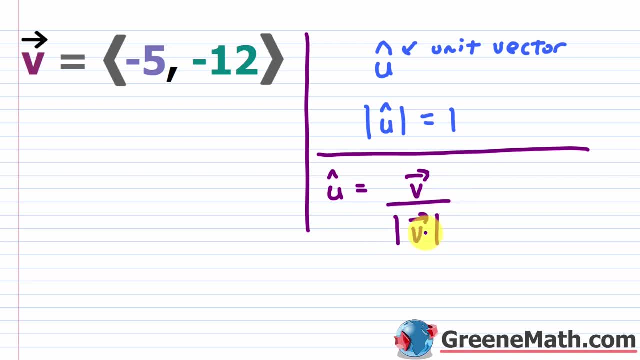 really think about this as multiple vectors. okay, So you can really think about this as multiple vectors. okay, So you can really think about this as multiple vectors. okay, So you can really think by a scalar one over whatever this is. So I'll further break this down and say: this is the vector. 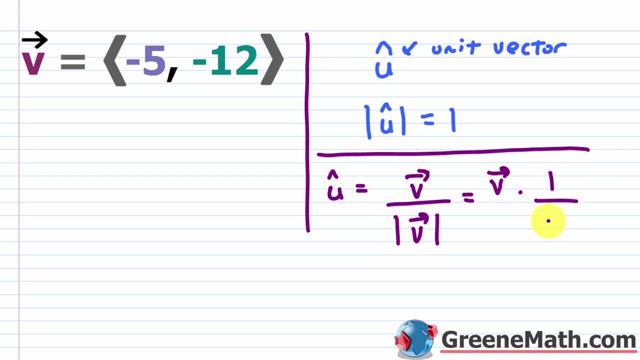 v times one over, whatever this result is. so the magnitude of this vector v. Remember, in the end this is going to be a number, right? This is some number, okay. So if I wanted to practice on this one, let's say this vector v- okay, has a horizontal component of negative five and a vertical component. 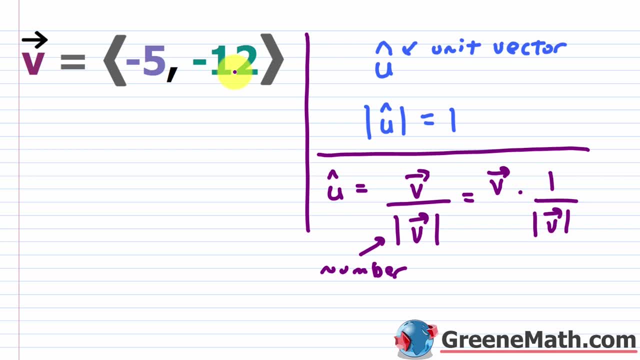 of negative 12,. how would I find the unit vector u in the direction of v? So basically in the, but now I have a magnitude of one. So what I would do is I would first find the magnitude of v. so the magnitude of v. Hopefully you remember that formula. You're going to take the square. 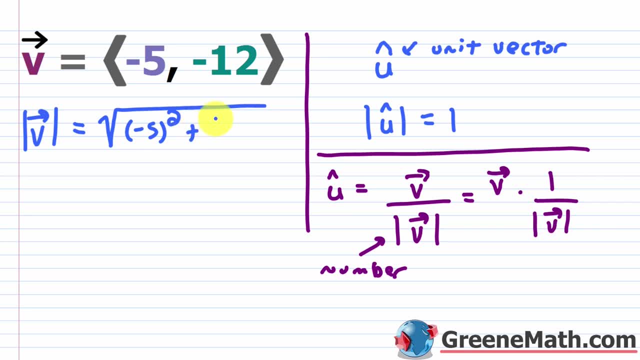 root of I'll have negative five being squared plus negative 12 being squared. So each one of these guys is going to be squared and you're going to find the sum of those two results okay. So I know, negative five squared is 25, negative 12 squared is 144.. So this would be my vector v. 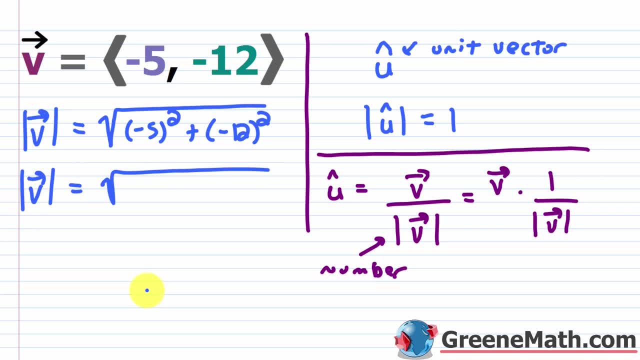 the magnitude of that guy would be: the square root of 25 plus 144 is 169, and the square root of 169 is 13,. right, So the magnitude of this vector v is going to be 13,. okay, So that's easy enough. Once you have this result, you can basically just: 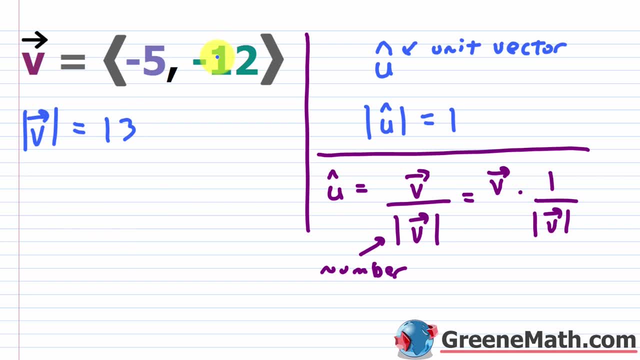 divide. okay, divide each one of these components by the magnitude of that vector and you're done. right, You've set up your unit vector u, okay, But if you want to kind of go about this the long way, let's just go ahead and use this formula here. So you have your vector v. I'm going to write it in. 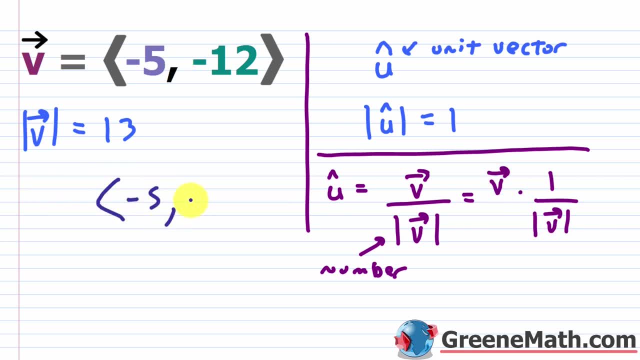 component form. So I'm going to say this is negative five squared, and I'm going to write it in component form: Negative five comma, negative 12, and let me make these a little bit wider, okay, So it's more consistent. So like that, and I'm going to multiply by one over the magnitude of that vector v, So one. 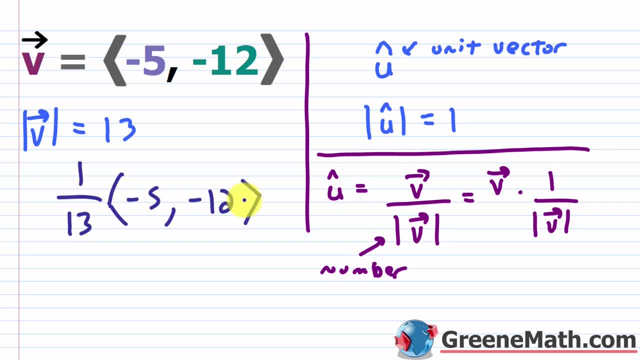 over. in this case it's 13.. So you can see, this is just a scalar multiple, right? So I can either multiply by one over 13,, or I can just divide by 13.. It doesn't matter, right? So in the end, 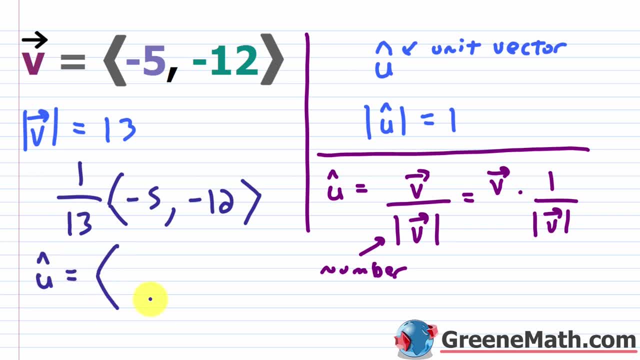 my unit vector u, okay, would be equal to in component form. you'd have negative five over 13. comma, negative 12 over 13,. okay, That's all you need to do. I want to prove a few things to you. One, that the magnitude of this vector u is one. 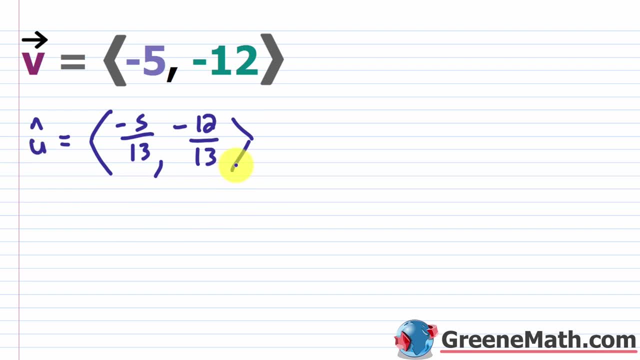 and also that the direction angle is the same. okay, So for the magnitude, again, it's very, very easy. So the magnitude of this unit vector u is going to be the square root of. so let's go ahead and say this is going to be negative, five over 13 being squared plus, you're going to have 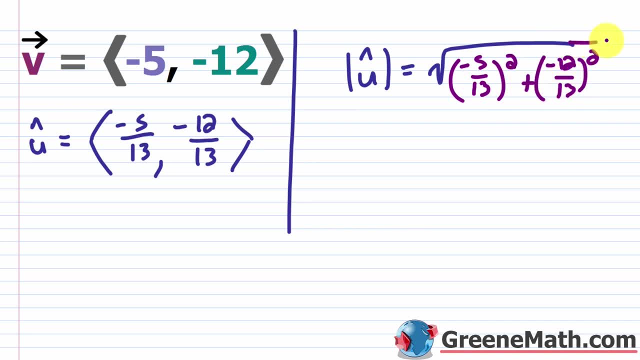 negative 12 over 13 being squared. okay. So negative five over 13,. if you square that negative five squared is 25, 13 squared is 16.. So let me write this down here: The magnitude of this vector u is going to be equal to the square. 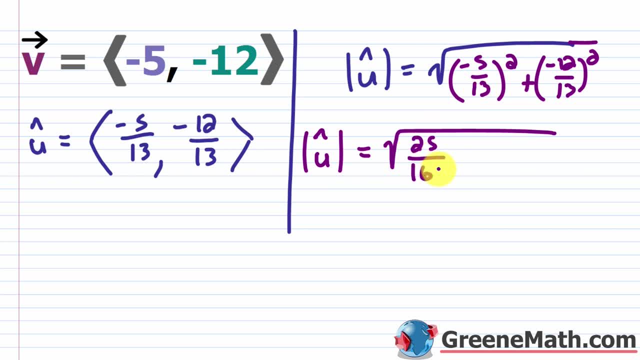 root of this would be 25 over 169, then plus negative, 12 squared is 144, and then 13 squared again is 169, okay, So if you add these guys, you have a common denominator: 25 plus 144 is 169.. 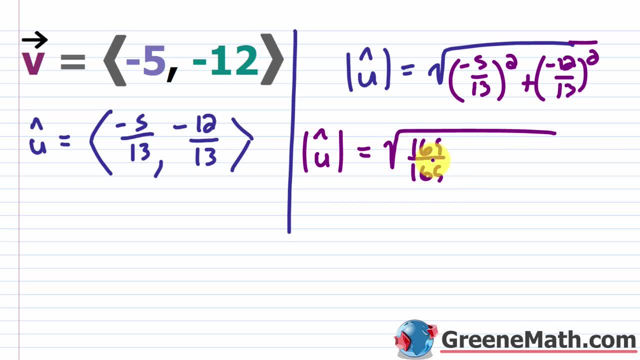 So you get the square root of 169 over 169.. This is obviously one and the square root of one is one, So you can see the magnitude of this unit. vector u is one. okay, So that part works out. What about the direction angle? okay, You're going to see that. basically, if you think about 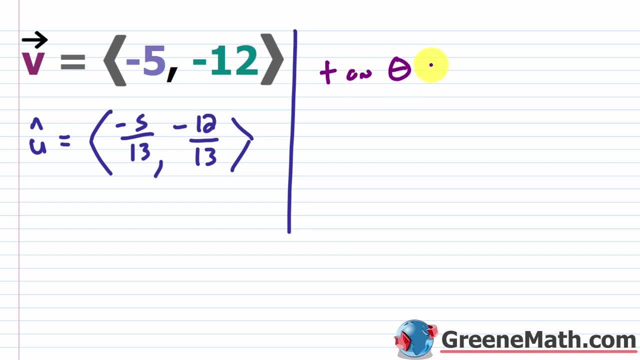 the direction angle, remember, the tangent of theta is going to be equal to this negative 12, okay, over this negative five, right, Which in this case you might as well just say it's 12 fifths, right. But again, we have to think about what quadrant we're in, because if we do the 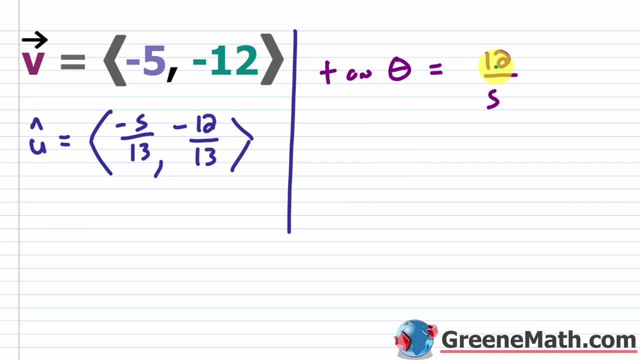 inverse tangent. okay, we're going to, in this case, because this is positive, we're going to get something in quadrant one. okay, But this is in quadrant three because we have a negative x value and we're going to get something in quadrant two. okay, So we're going to get something in quadrant three. 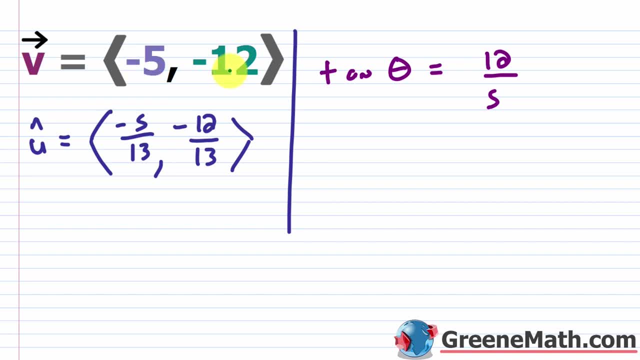 and a negative y value. So I go to the left and I go down, so I'm in quadrant three. So what I want to do here is say the inverse tangent. the inverse tangent of this 12 fifths here would be equal to- or let's say approximately, because we've got to punch this into a calculator I get. 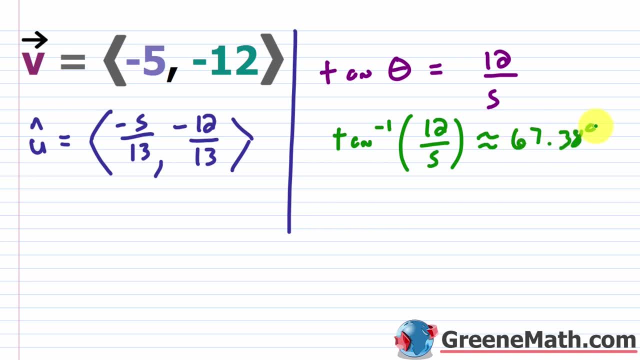 about 67.38 degrees. okay, And because we're in quadrant three, we want to add 180 degrees to this. okay, to get our measurement for theta okay. So we'll say theta is approximately. I'll say 247. 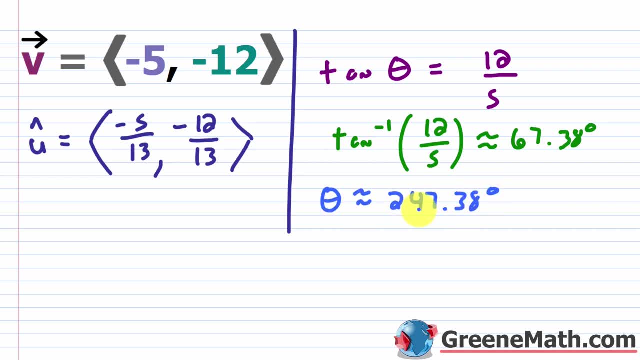 point 38 degrees. okay, So this is your direction angle. You already know how to find that. Now, if you look at it for this unit, vector u, you'll notice you're still in quadrant three. right, This is negative and this is negative. okay, So you're still in quadrant three and I want you to think. 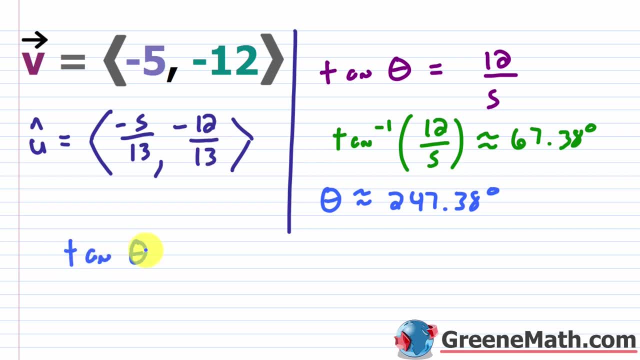 about the fact that you still have tangent of theta is equal to now. it would be negative 12 over 13,, divided by negative 5 over 13.. Well, the negatives are going to cancel, right? So you'd have 12 over 13.. So you'd have negative 5 over 13, and you'd have negative 5 over 13.. So you'd have. 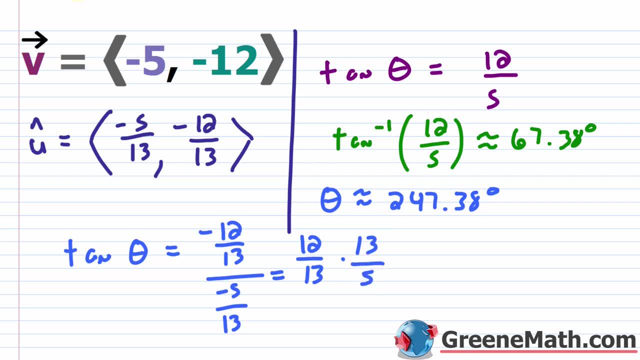 times flip this guy 13 over 5, okay, And the 13s are going to cancel. so I'm back to this 12 fifths, right? So the tangent of theta is equal to 12 fifths and again I'm still in quadrant three. 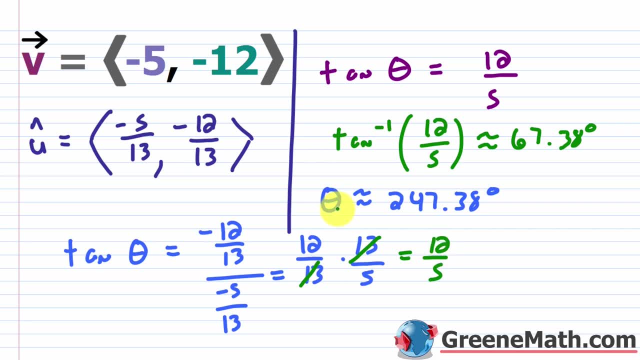 so I go through the same steps and I'm going to end up with a theta here. okay, my direction angle, which is again approximately 247.38 degrees. So you see that we've set up this unit, vector u, that has a magnitude of one, and it's in the direction of our vector v. All right, let's change. 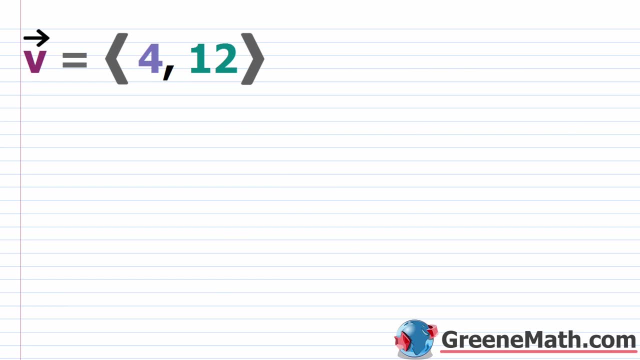 that. So sometimes you'll be asked to find a unit vector u, basically in the opposite direction of some vector v. So all you really need to do here is think about the concept of: well, if I multiply a given vector by negative one, it's just that vector that has the opposite direction. okay, Same. 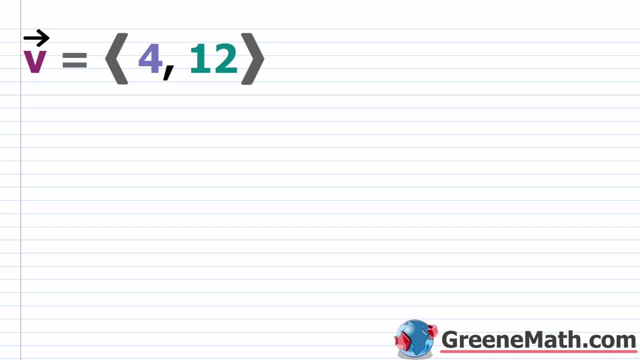 magnitude, but an opposite direction. okay, So we're going to use that concept here and just multiply our regular answer by negative one. So in other words, I would have my unit vector u is going to be equal to. we'll have this vector v and then I'm going to have my unit vector u. 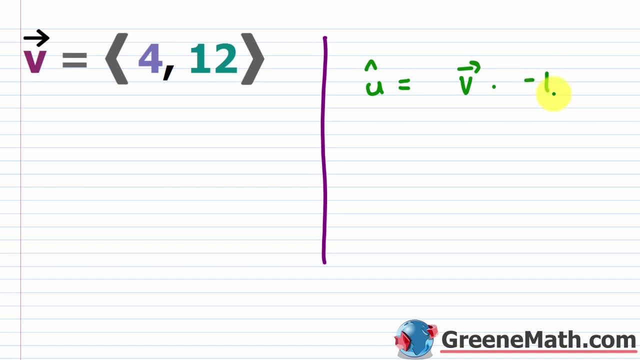 times. what I'm going to do here is put negative one, okay, instead of positive one. so negative one over the magnitude of this vector v. So let's go ahead and find the magnitude of our vector v. So the magnitude of this vector v is going to be equal to the square root of. so four squared is: 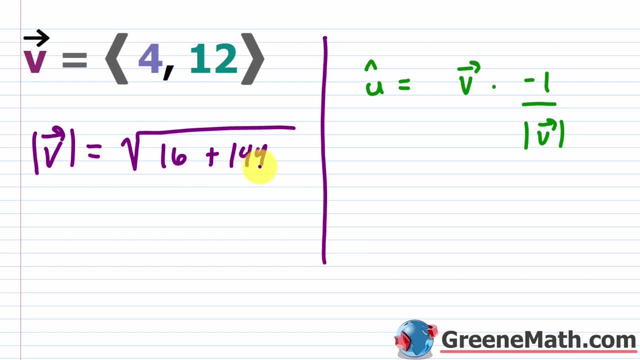 16, plus 12 squared is 144.. If you add these guys together, you get 160.. And what I can do is I can factor this and say: this is 16 times 10, okay, 16 is a perfect square, So this would be four times. 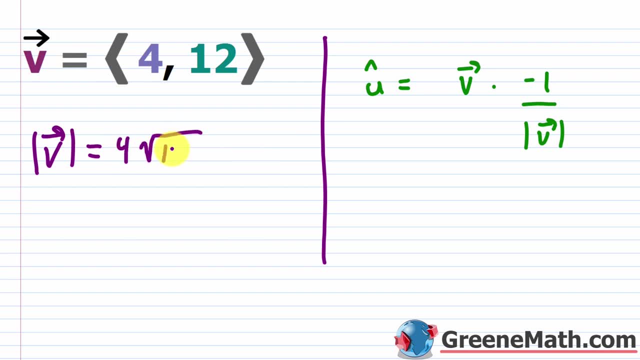 the square root of 10,. okay, So I'll say this is four times the square root of 10.. Now all I'm going to do here is either divide everything by the negative of this guy right here, or you could say, multiply by negative one over that guy. whatever you want to do, I'm just going to make. 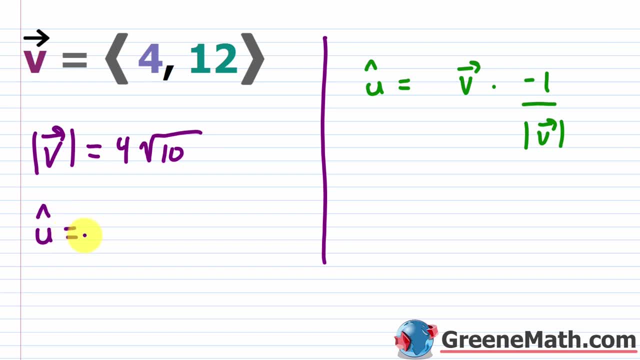 this a little bit quicker and say: my unit vector u that I'm looking for in this case is going to be: I'll take the four, okay, And I'm going to divide it by the negative of four times the square root of 10,, okay. And then let me put my angle brackets in here, and then I'll have my 12, and then I'm. 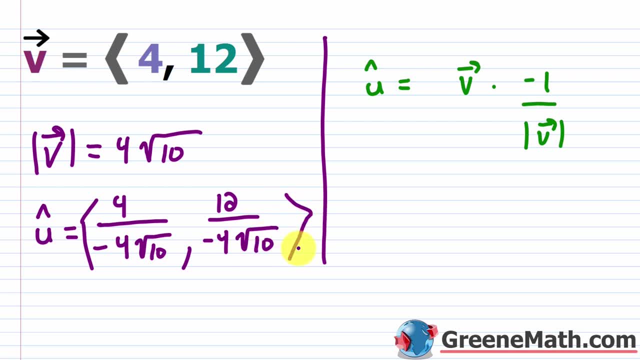 going to divide that by the negative of four times the square root of 10, okay. And then I'm going to negative of four times the square root of 10, okay. If I didn't ask you for the opposite direction, this would be positive one, But since I did, it's a negative one there. So that's why these are. 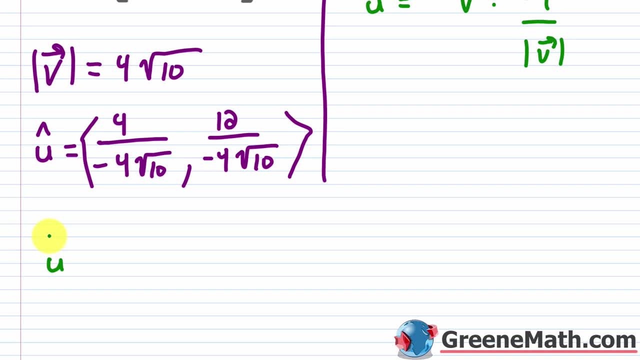 negative here. okay, Let me get some room going here. So let me go ahead and set this up as the unit vector u is equal, to put my brackets there. So we know we're going to have to rationalize the denominator there. So four divided by four is one. So let me put a negative out in front. Let me put 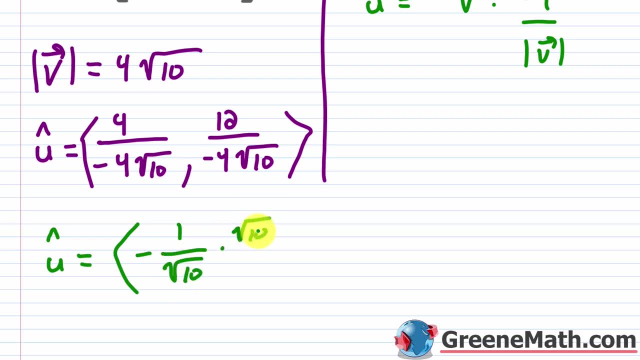 a one over the square root of 10.. And I'll just multiply this by the square root of 10 over the square root of 10 to get that out of the way. So this becomes 10. down here, Okay, And up here, this is the square root of 10.. Okay, So this is the square root of 10.. Now 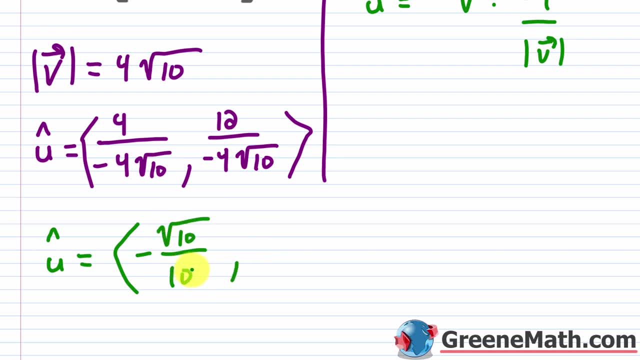 it is common to not rationalize the denominator for these examples. It's really up to you or your teacher. Just get with them and see what they want you to do. For this one, we have 12 divided by four, which is three, And of course you have the negative. So let me go ahead and put. 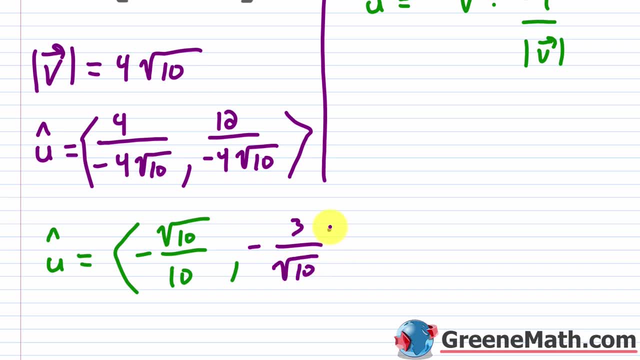 three over the square root of 10.. And again I'm going to rationalize the denominator: So times the square root of 10 over the square root of 10.. Okay, So we're going to multiply by that, So in the numerator I'd have three times the square root of 10.. So three times the square root. 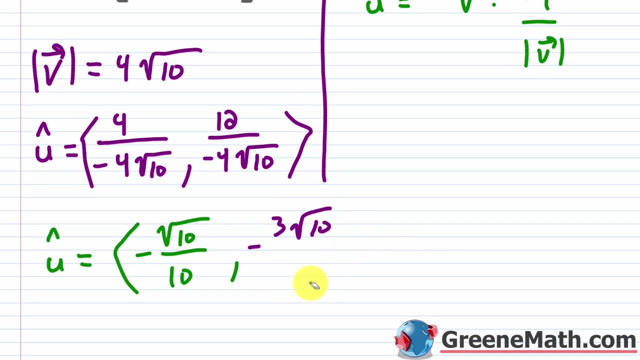 of 10.. In the denominator I would have 10.. Right, So basically the way this guy would work is: you would have this unit, vector u, which again is in the opposite direction of my vector v. the horizontal component is negative square root of 10 over 10.. And the vertical component is: 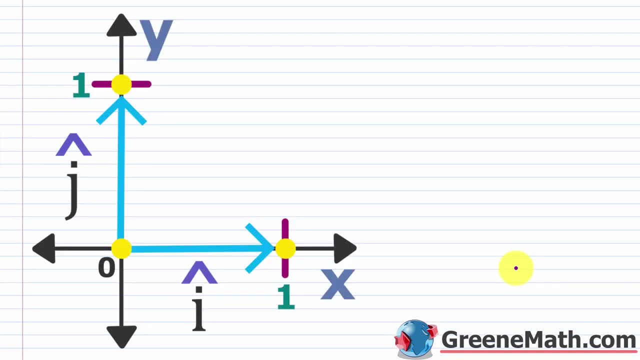 negative three times square root of 10 over 10.. All right, so let's continue to talk about these unit vectors, And now you're going to see these two extremely useful unit vectors, which are defined using this i and also this j: Okay, 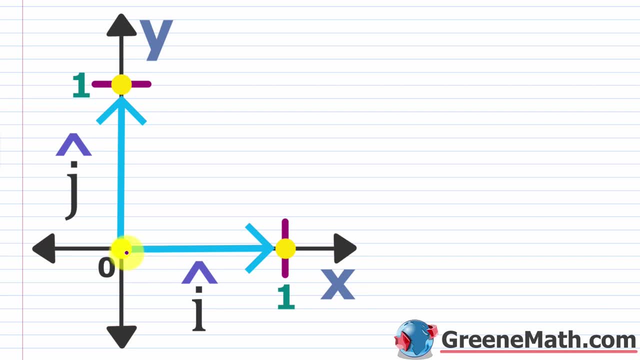 So you see, on the screen here we have this little graph, you have a directed line segment that starts at zero comma zero, okay, and ends or terminates at the point one comma zero. So the initial point is zero comma zero, or the origin, the terminal point, is one comma zero. So we have 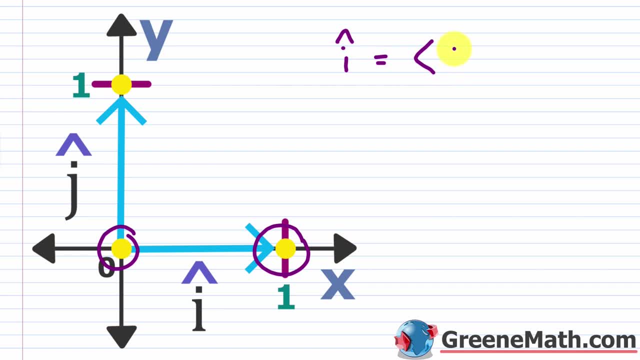 this unit vector i. okay, in component form, this is one comma zero, like this: okay, this is not the imaginary unit i, So please don't get confused by that. Then, similarly, we have this guy that is denoted with a j. So we have this guy that is denoted with a j. So we have this guy that is: 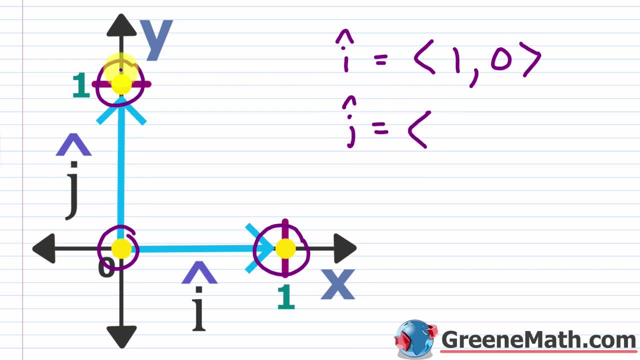 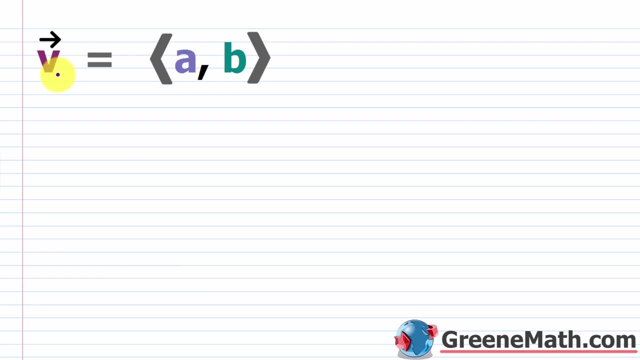 denoted with a, j. So we'll say j here with my little hat. So this guy, it terminates at zero comma one, okay, And basically we're going to use this guy to rewrite something like this: So our vector v, in component form we have a comma b, okay, But using those two vectors, i and j. 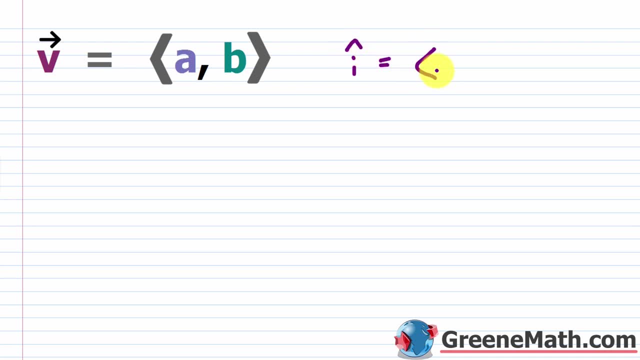 basically what you can do again, because the vector i in component form is one comma zero, okay, and the vector j in component form is zero comma one, you can take your horizontal component and multiply it by this guy. So let's say the vector v. I could also define it saying it is: 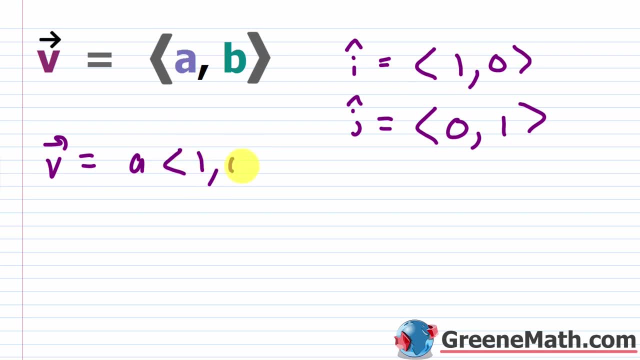 this: a multiplied by this: one, comma zero. okay, then plus- and I probably need to move this down a little bit- So plus this b here, multiplied by this guy: zero, comma one. okay, So you know that these are just scalar multiples. at this point, if I multiply through, this is basically a comma zero. 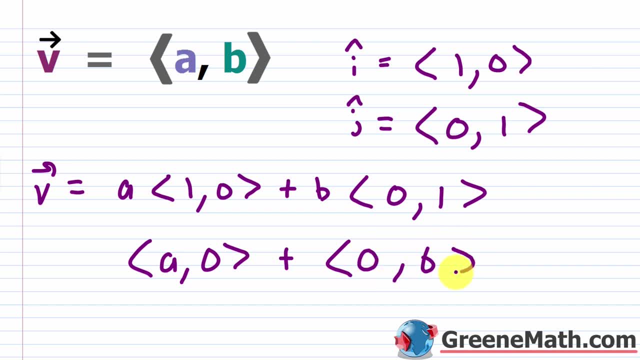 okay, plus this is zero comma b, okay, And then if I add these two together, I'm right back to what I started with. So I didn't do anything legal. Now, what you can do at this point is just replace in each case this with the unit vector i. 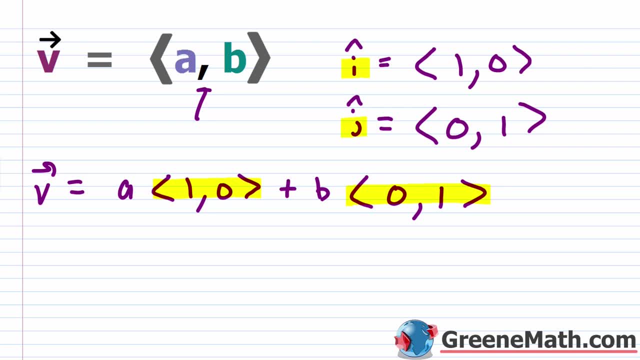 and this with the unit vector j. okay, that's all you're going to do. This is called writing it in the i comma j form, or you might hear it as a linear combination of the standard unit vectors i and j. okay, So I'm going to say the vector v. now it's going to be written as a times: the. 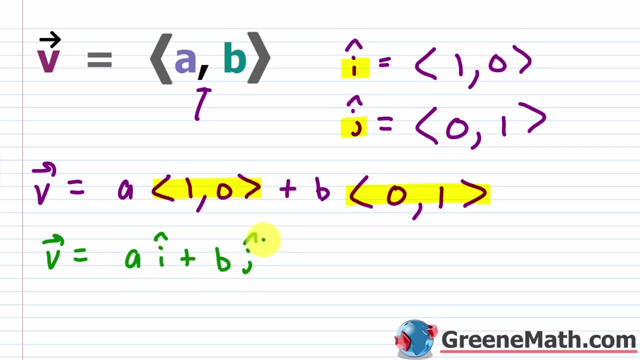 unit vector i plus b times the unit vector j. okay, So if you see something in this form, to put it in component form, basically again, the vector v is what It's, just in component form. this is your horizontal component, right and then comma. this is your vertical component. 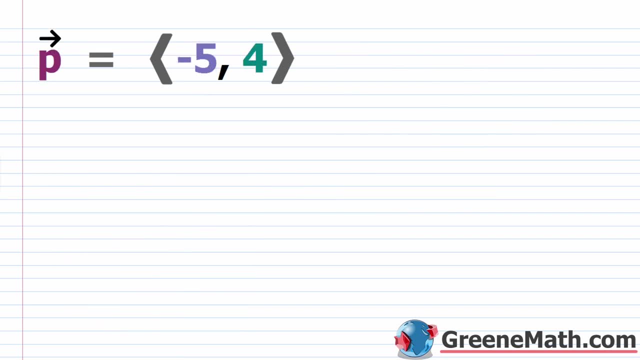 that's all it is okay. If we look at a little example here, let's say I have some vector p and I want to write it as a linear combination of those two standard unit vectors, i and j. all I'm going to do, I'm going to say: this guy p, this vector is negative five. 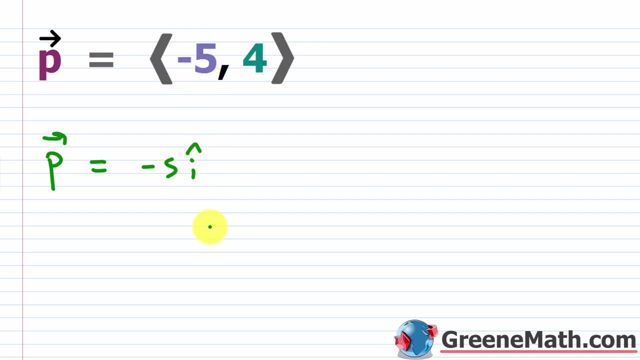 this is the horizontal component multiplied by this unit vector i. okay, then plus this guy, four, okay, multiplied by that unit vector j. that's all it is. Again, if you go back through this the long way, all you're really saying is that this vector p is. 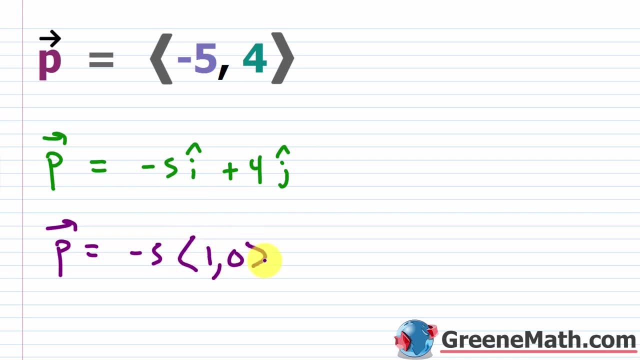 equal to, you'll have negative five times. this is what? one comma zero. then plus four times, this is zero comma one. and again, all I'm doing is- if I kind of move this up here because I'm going to run out of room- this vector p is what? Now it's negative five. okay, comma zero. 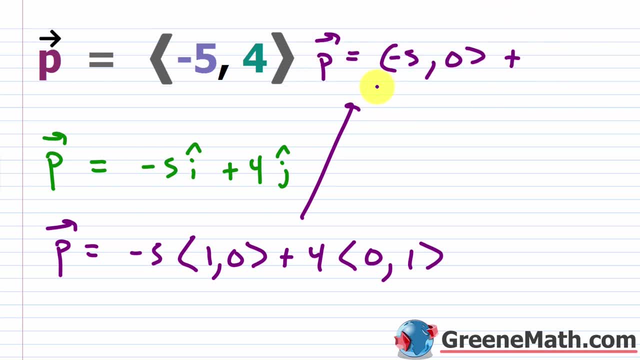 plus- and let me move this down a little bit so I can fit everything. let me change this up because I'm getting sloppy with my notation there. so, plus over here, this would be zero, comma four again if you add these guys together. 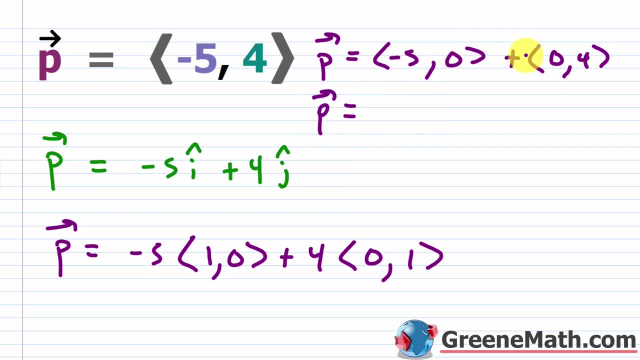 this vector p is back to what it started with, right, this is going to be negative five plus zero, which is negative five, and then comma zero plus four is four. okay, so it's just two different ways to write the same thing. this way, right here, you're going to see a lot. 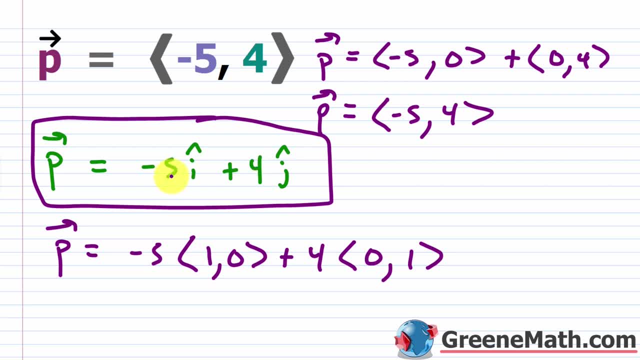 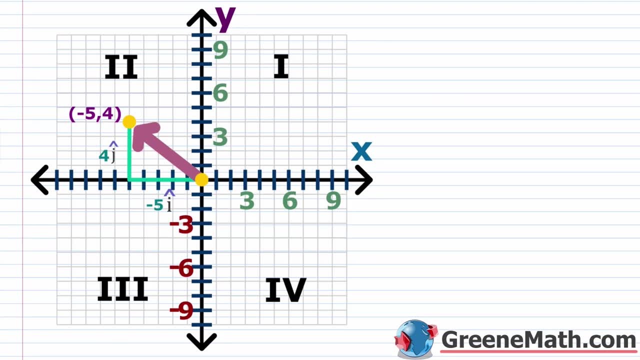 okay. so you need to know how to go back and forth between the two if you wanted to graph something like this. the terminal point is going to be at negative five comma four. so if we looked at this on our little coordinate plane, here again the horizontal movement here. 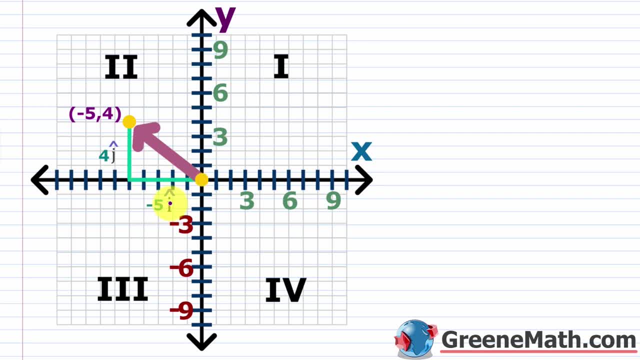 is given by the negative five times this unit vector. i okay, it's just basically like if I said the horizontal movement here is given by this negative five comma, zero right, and let me make that a little bit better. so basically, if I started here and I went five units to the left, 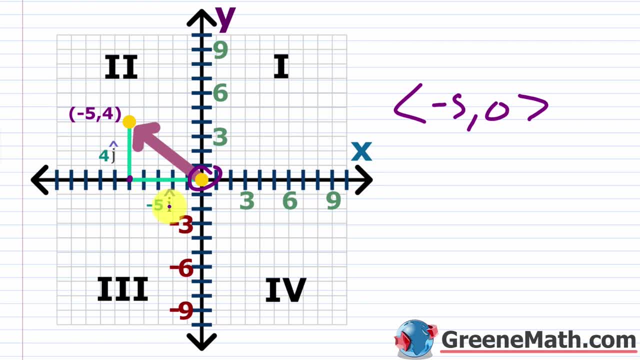 end up right there. okay, that's my horizontal movement, given by this negative five times the unit vector i. then for the vertical movement, if I'm starting here and if I go up, well, basically this is given by four. 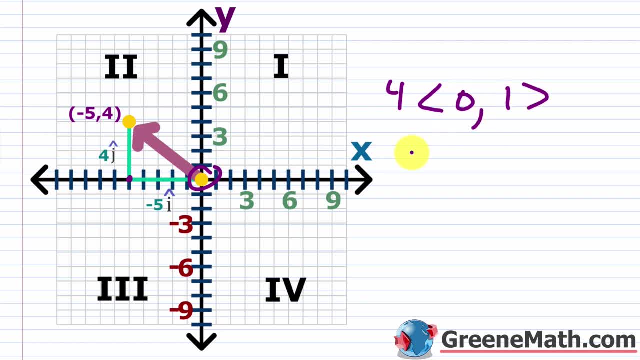 times the unit vector j, right, four times that zero comma one like this. so this is zero comma four, right, I'm just moving up four units vertically. so when you put those two guys together you end up with this directed line segment with a terminal point at negative five. 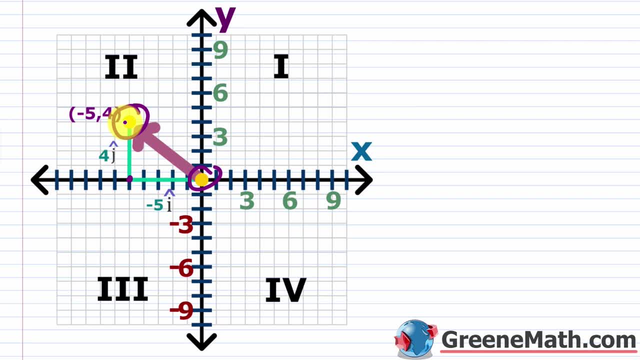 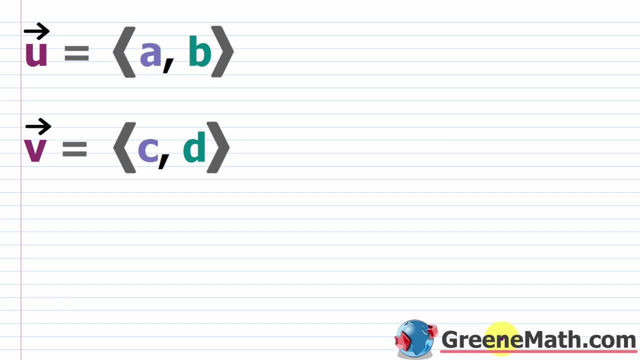 comma four: five units to the left, four units up, so that's all. it is all right. let's talk about something called the dot product now, and this is going to lead us into a topic called finding the angle between two vectors. okay, so we start with the dot product and the dot product of two vectors. 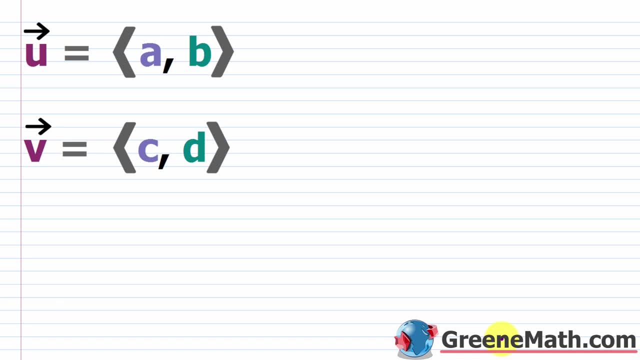 is going to be a real number. so we're going to start with the dot product and the dot product is going to be a real number, so this is not going to be a vector. this is also called the inner product, okay, so someone might refer to it that way. now the dot product for us is going to be: 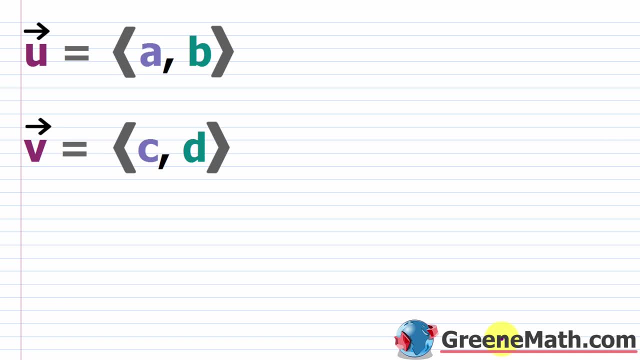 used to determine the angle between two vectors, and we'll get to that shortly. so when you have the dot product of two vectors, let's say u and v. so I have u and v, those two vectors. I'm going to write the vector u, then dot the vector v. okay, so this is the dot product and basically. 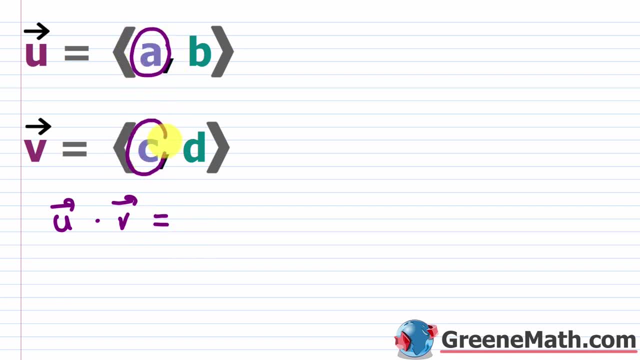 all I'm going to do is I'm going to multiply the first component here by the first component here, so a times c. so in other words, horizontal component times horizontal component. then plus second component here times second component here. so vertical component here times vertical. 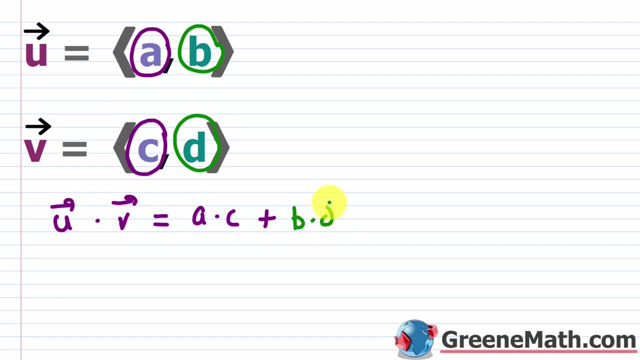 component here. so b times d. it's a very easy pattern to remember. once you do a few examples, it just becomes second nature. okay, so let's look at an example. so we want to find the dot product of this vector u and this vector v, so you're going to do the vector. 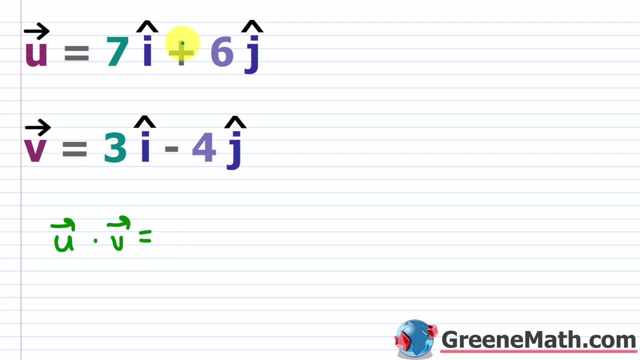 u dot the vector v like this. and again, if this is confusing for you because you're going to go to the antisocial v, you're going to write it. see that V is square root of Squares, average лю, which is exactly W. don't worry, because again it's as this, linear. 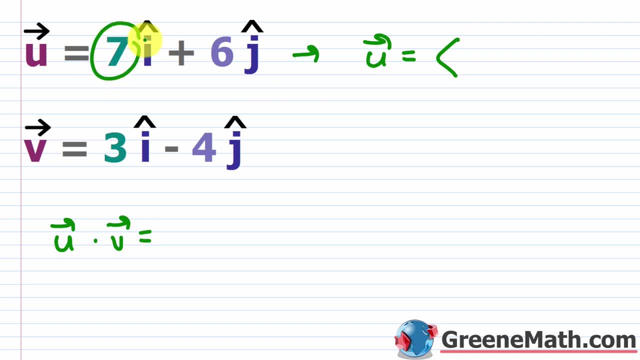 combination of the unit vectors I and J. you can always put it in component form. so the vector u is again in component form. this is my vertical component. okay, do this a few times and then it becomes very easy, right? so the vector v. this is my horizontal. 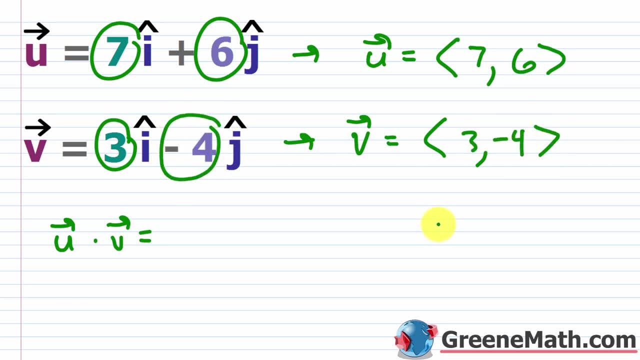 component this and the whole thing with the negative. so let me make sure I do that properly. this is your vertical component, okay. so either way you want to do it, but so first times first, then plus six times negative four, so second times second, so six times. 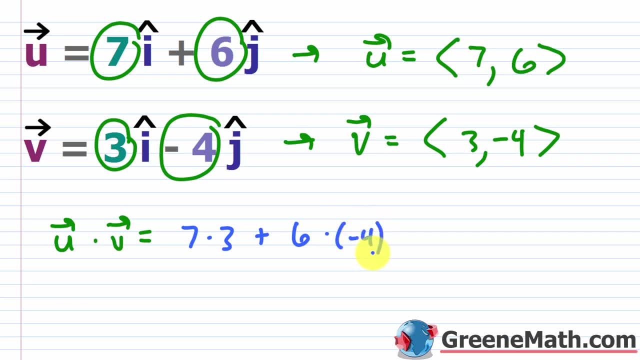 negative four. That's all you're doing. okay, Just match things up and say these guys are being multiplied, and then these guys are being multiplied. That's all you got to do. So once you have this set up, seven times three is 21,. then basically, plus six times negative four is: 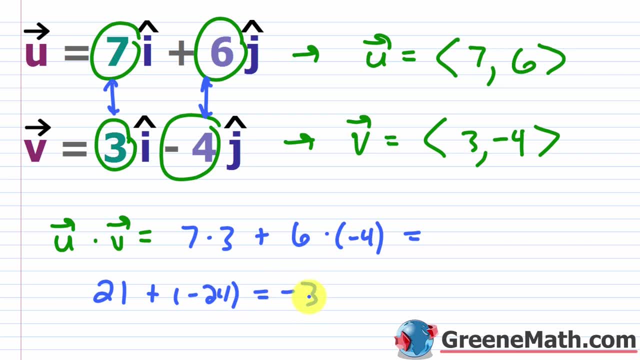 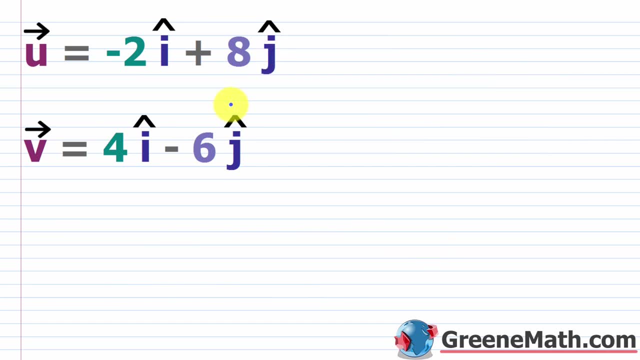 negative 24.. So this would be negative three. So that's your dot product of this vector u and this vector v. Okay, let's look at another example. If you want to pause the video and put these in component form, that's up to you. I think you can get it like this. So the vector u is: 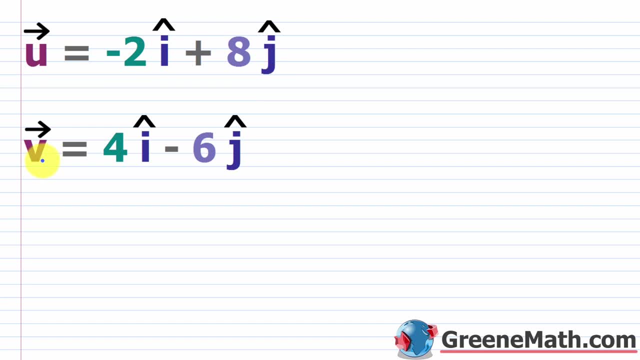 negative: two times the unit vector i plus eight times the unit vector j. Then this vector v is four times the unit vector i, minus six times the unit vector j. So the dot product of this vector u and this vector v, so u dot v would be what You're going to have. this guy times this guy. 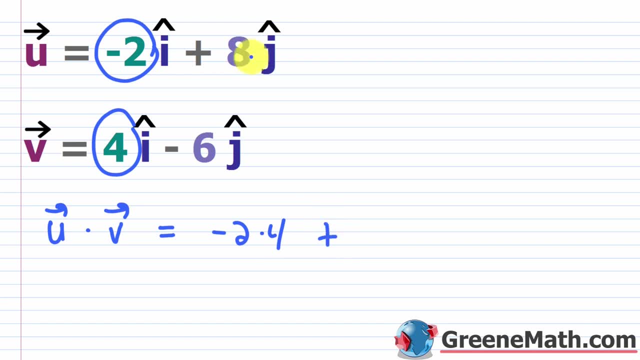 right. So first times first negative, two times four, then plus this guy times this guy. So eight times negative six, eight times negative six, And again, if something's negative, make sure you take that with it. Okay, so let's put equals here. 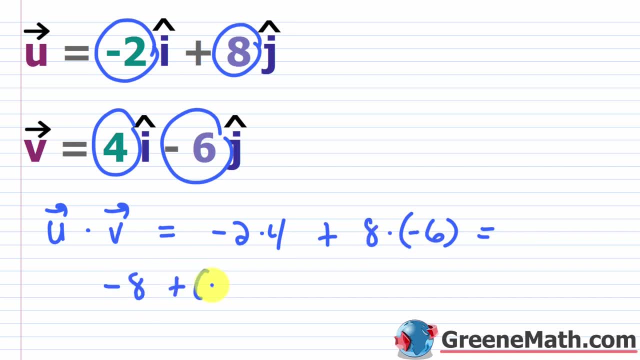 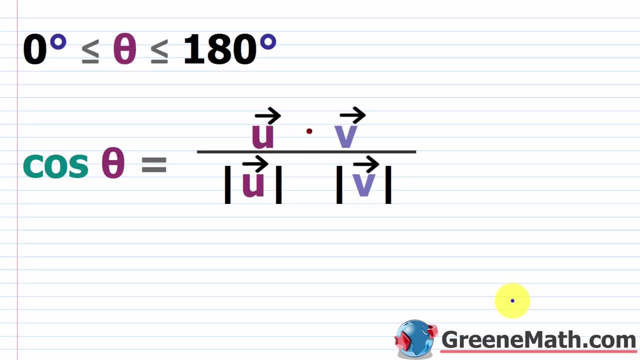 Negative two times four is negative eight, And then plus eight times negative six is negative 48. And of course, this is really easy: This is just going to be negative 56.. All right, so now that we understand how to find the dot product of two vectors, we're going to use this. 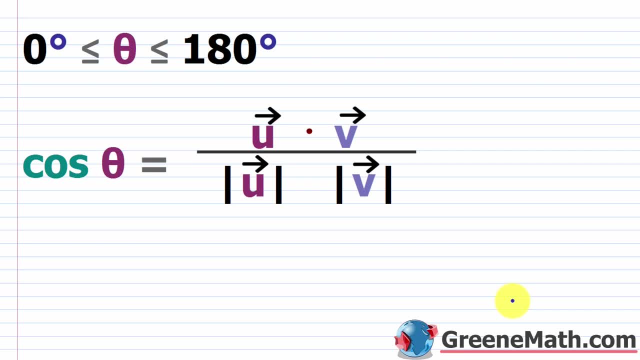 now to find the angle between two non-zero vectors. So let's suppose we have these two non-zero vectors, Let's call them u and v, Okay, and we want to find the angle between them And we'll say theta. So we'll say that theta is greater than or equal to zero degrees, and also less than or. 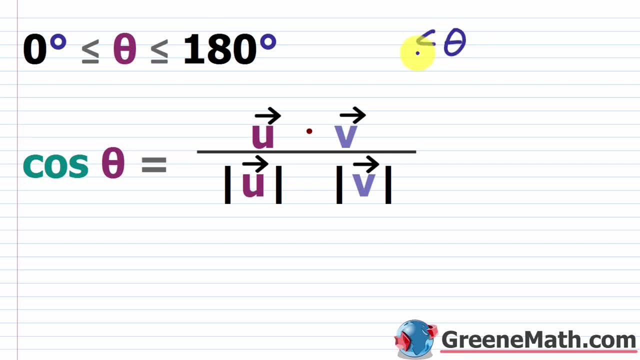 equal to 180 degrees. Or we could say theta is greater than or equal to zero and less than or equal to pi, if you want to work with radians. So we can come up with this little formula here. This is derived from the law of cosines, So we have the cosine of this angle. theta is equal to. 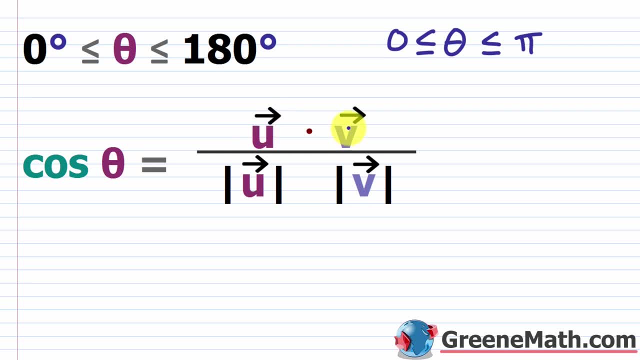 the dot product of this vector u and this vector v over you have the magnitude of your vector u times the magnitude of your vector v. Okay, so that's all it is. If you want to find theta, you're going to use your inverse cosine. 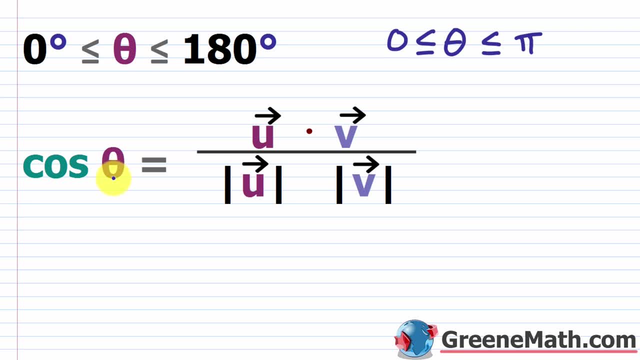 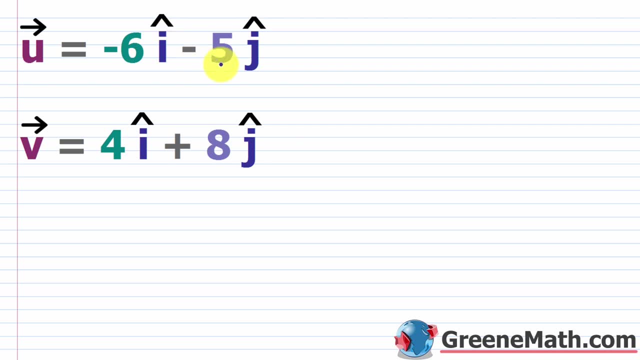 function. Okay, you're just going to be punching this stuff into a calculator, So really really easy. All right, let's look at the first example. We have a vector u- okay- which is negative, six times the unit vector i minus five times the unit vector j. Then we have this vector v, which is four. 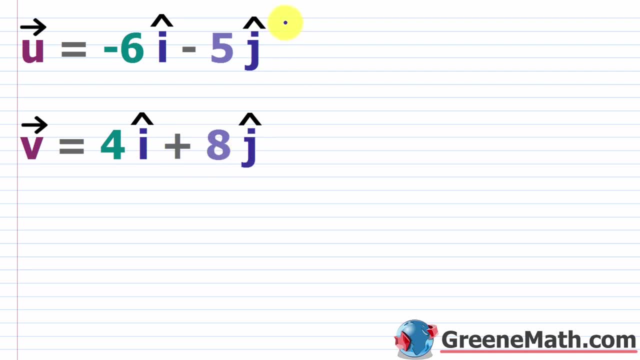 times the unit vector i plus eight times the unit vector j. Okay, so if I want to basically set this guy up, first and foremost, if you're still confused by these linear combinations of the unit vectors, you can always write this in component form. okay, to ease your confusion Again, all I'm going to do 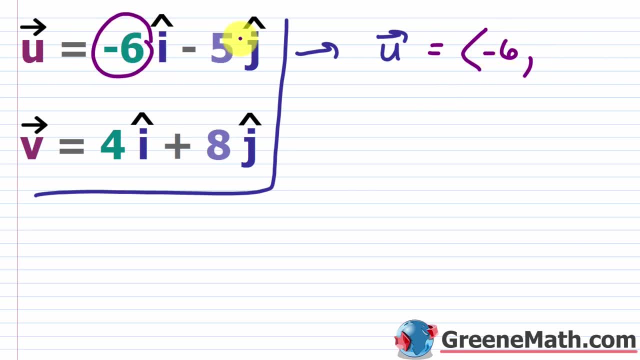 to do. that is, take this guy as a horizontal component, okay, and then this guy is the vertical component. That's all I'm going to do. So if you're confused at this point, just do that for a little while, and then eventually this will click for you. So then this guy for the vector v. 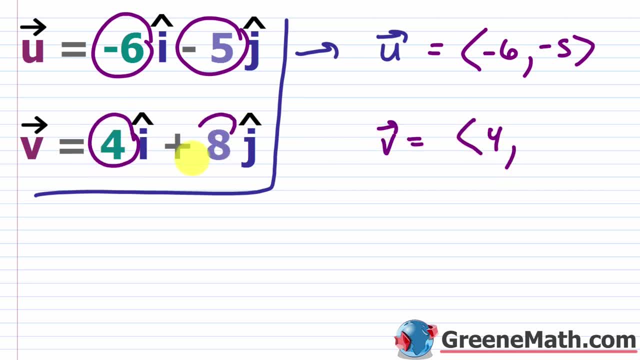 in component form it's going to be four comma, then you're going to have eight. Okay, that's all it is. So if I want my dot product, okay, so the dot product of this vector u and this vector v. 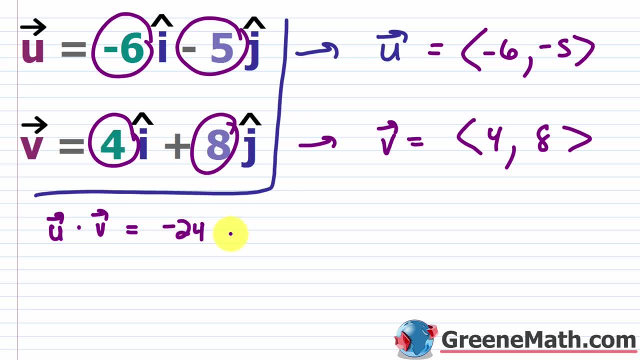 this is going to be what Negative six times four, that's negative 24, then, plus negative five times eight, that's going to be negative four. Okay, so this gives me negative 64.. Then if I want the magnitude of this vector u, okay, this is going to be the square root of, so I'd have 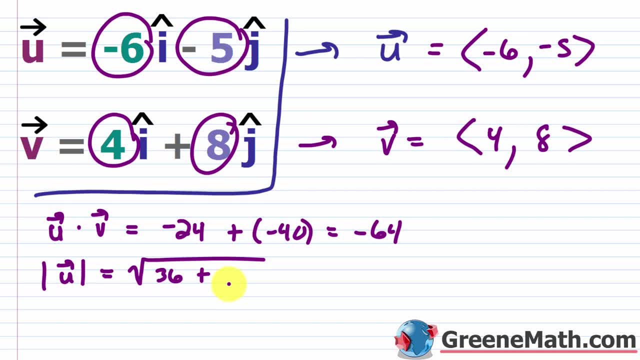 negative six squared, that's 36, and then plus negative five squared, that's 25.. So this would be the square root of 61.. Okay, then the magnitude of this vector v. let me change my ink color here. this is going to be the square root of four squared is 16, and then eight squared is 64.. 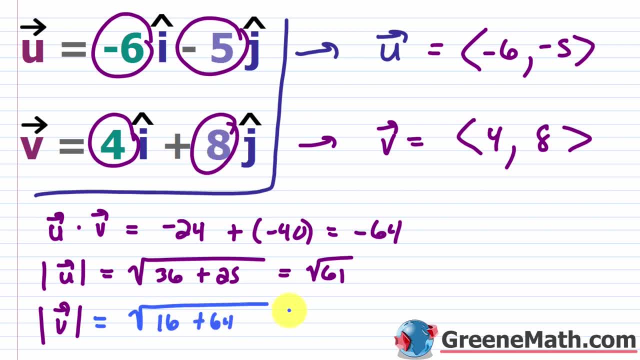 So 16 plus 64 would be the square root of 80.. You could simplify that if you wanted to. Again, you're punching this stuff into a calculator, so if you're trying to save time, I wouldn't even worry about it. But since this is a math tutorial, I'm going to take the extra step and write this: 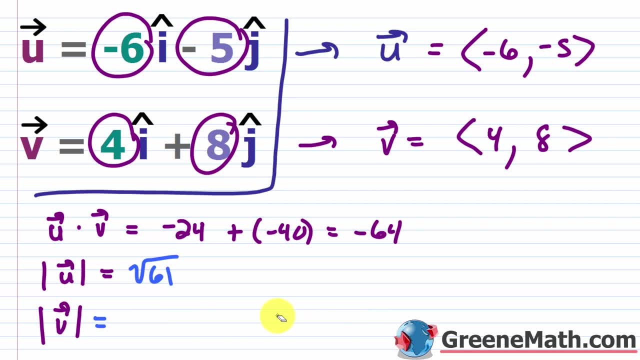 down here. Let me just put this as a square root of 61.. Let me write this instead of the square root of 80,. let me say that 80 is 16 times five and 16 is four times four. right, So I'm going to. 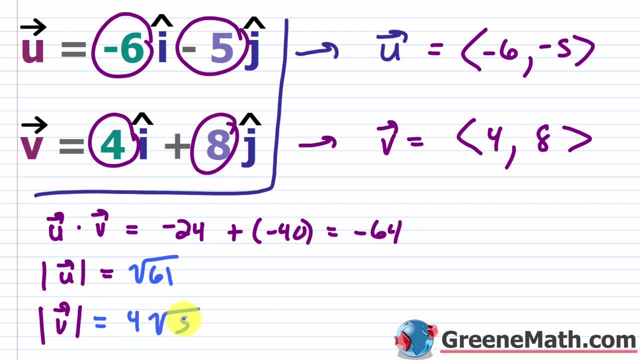 say, this is four times the square root of five. right, Because 16 is just a perfect square. Okay, so now we have everything we need. Let me tighten this down and put negative 64 here. Hopefully you have this copied down. I'm going to get rid of it because I need the room. 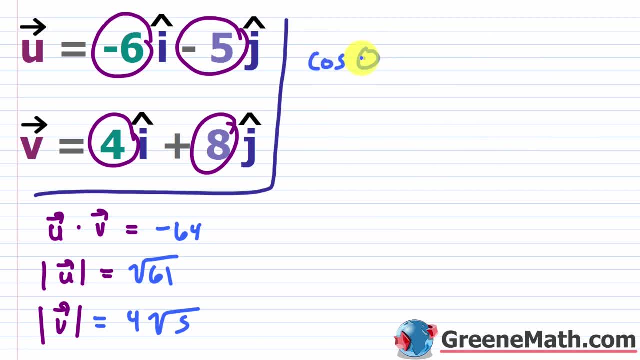 And I'm basically going to write my formula here. So the cosine of theta is equal to, again, the dot product so of this vector u. so the vector u dot the vector v, And then this is over the magnitude of this vector u, and then this is multiplied by the magnitude of this vector v. 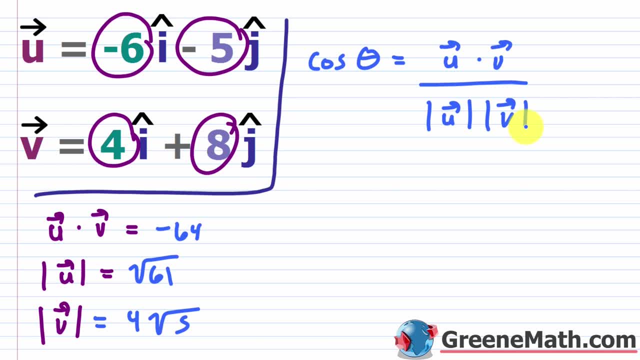 okay. So what I would do here is just plug in to the calculator and essentially you're going to say that theta is equal to the inverse cosine of all this, right? So your dot product of the vectors u and v. so this is going to be negative 64. Then over you're going to have the product of these: 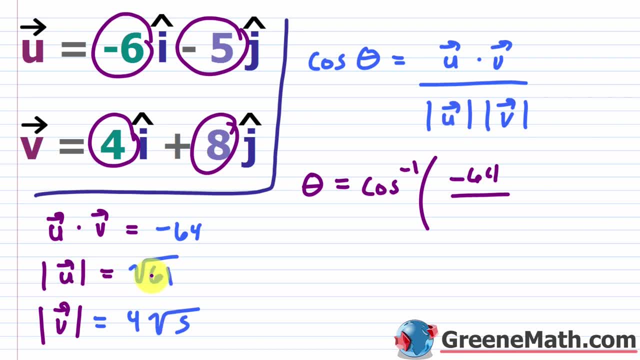 two magnitudes. So the magnitude of vector u is square root of 61, and then the magnitude of vector v is four times square root of five, So that would be four times the square root of 305,. okay, And again, you don't have to write all this out. If you're using a calculator, just punch it into it. 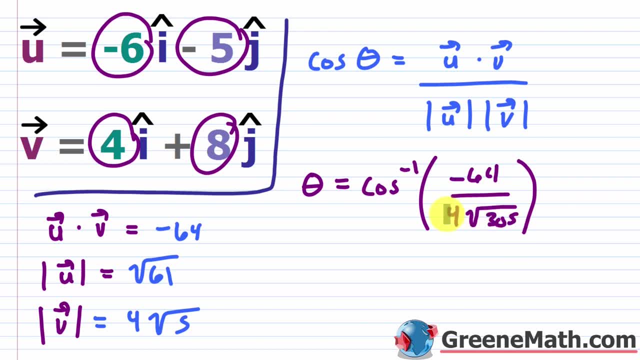 and you're done, But you might want to consider the fact that you should put parentheses around this guy when you punch it into your calculator. If you keep getting the wrong answer, that's usually what's going on. It just depends on your calculator, okay, So what I would do is punch this guy into the calculator as the argument for. 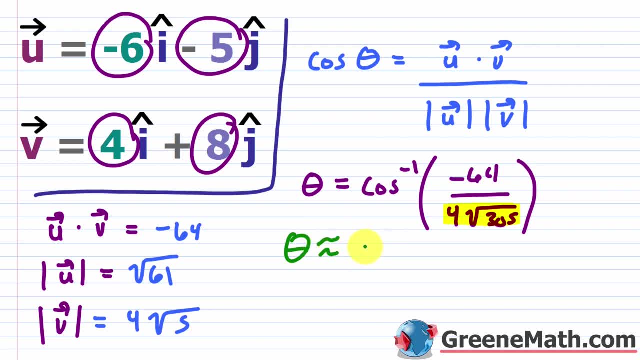 the inverse cosine function and I'll say theta is approximately 156.37 degrees. okay, So that's basically all you're going to do. And again, if you keep getting the wrong answer with your calculator, if it says something like domain error or something like that, then make sure you wrap. 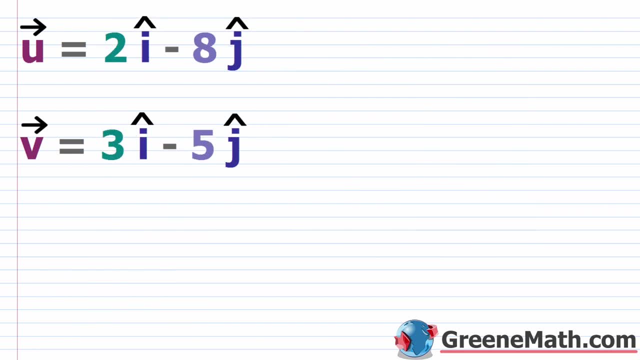 that right here inside of parentheses, and that should clear that up for you. Okay, Let's take a look at another one. We should know the formula at this point. Let me go ahead and do the dot product first. So the dot product of u and v. so u dot v. here is going to be what Two times three, which. 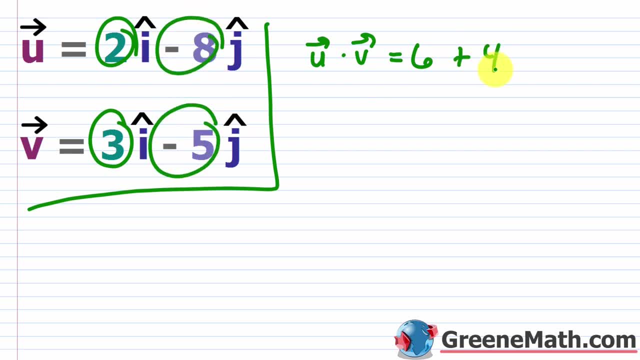 is six, plus negative, eight times negative five, which is going to be 40.. So this is 46,. okay, And then basically the magnitude of this vector u is the square root of you have two squared, which is four, then plus four, which is four, which is negative eight times negative five, which is going to be 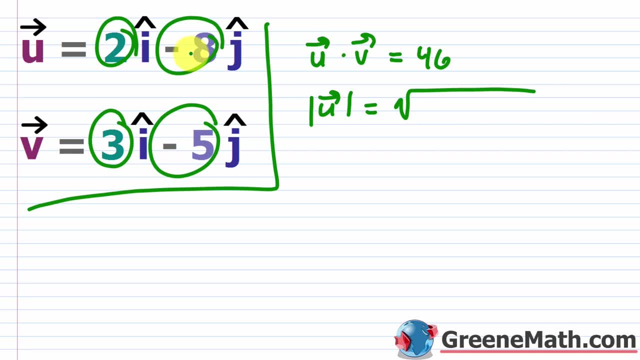 plus you have negative 8 squared, which is going to be 64.. So 4 plus 64 is 68, right, So square root of 68, again, you could simplify that at 17 times 4.. So it's technically 2 times the square root of. 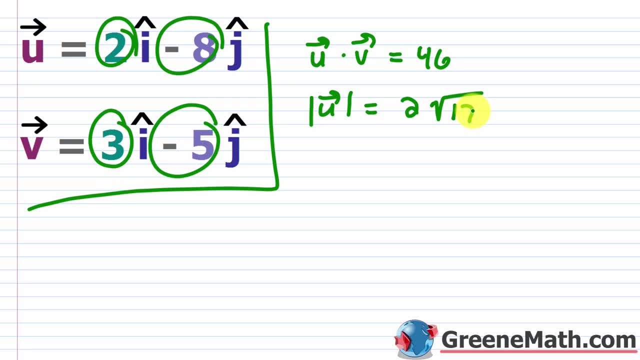 17.. Now again, if you punch this into a calculator, you know who cares, but I'm just writing this down for the sake of our tutorial. Okay, Now the magnitude of the vector V. we're going to have what You have. the square root of 3 squared is 9, then plus negative 5 squared is 25.. So this is: 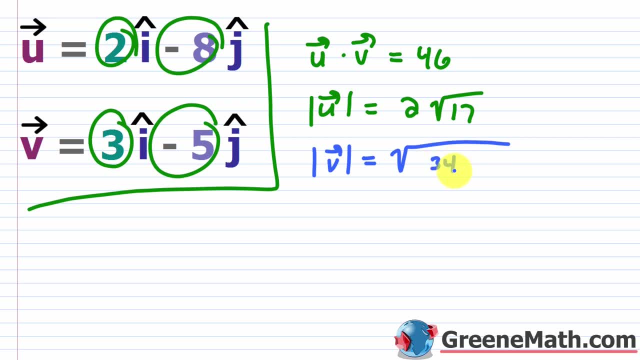 going to be square root of 34.. Now you can't simplify the square root of 34.. So let me erase this. I'm going to write this as the square root of 17.. Okay, Let me write this like the square 17 times the square root of 2, like this: Okay, So let's punch into the calculator. First, let me do. 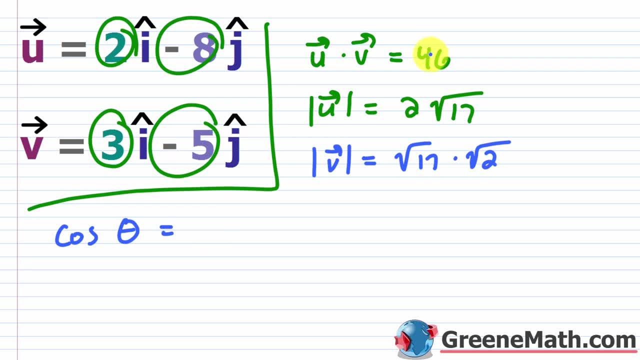 this cosine of theta is equal to. again, you've got your dot product, which is the u dot v. Okay So the vector u dot the vector v over you've got the product of these two magnitudes, Okay So the. 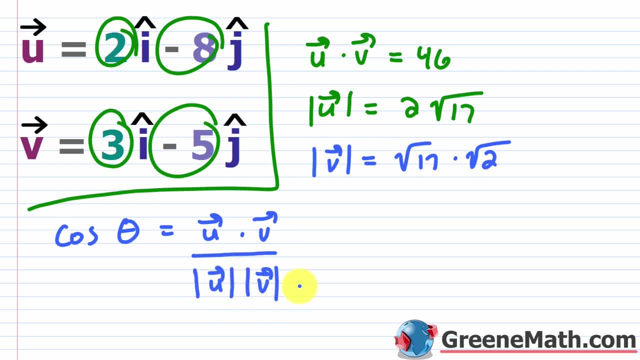 magnitude of this vector v is going to be the square root of 34.. Now, you can't simplify this vector u times the magnitude of this vector v. Okay, And then if I plug in to my calculator, what I want to do is say: theta is equal to cosine, inverse of all of this. Okay, So the dot product. 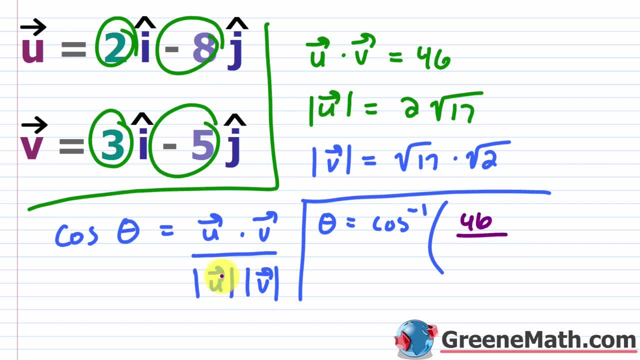 of u and v is 46 over, you're going to have the magnitude of u times the magnitude of v. So essentially what you have is 2, okay. times square root of 17. times square root of 17 is 17.. 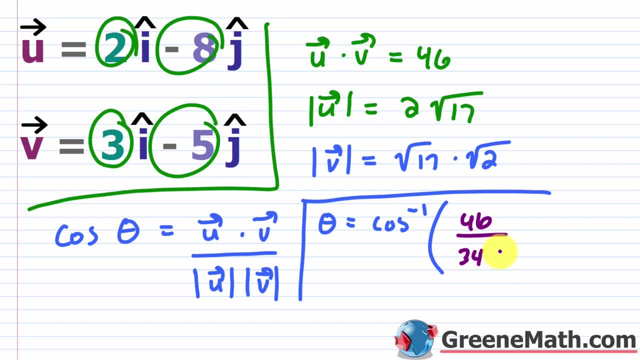 Okay, So that's just going to be 34.. Okay, And then times the square root of 2.. Now again, you don't have to go through all this. If you were writing this out on a test, you might want to. 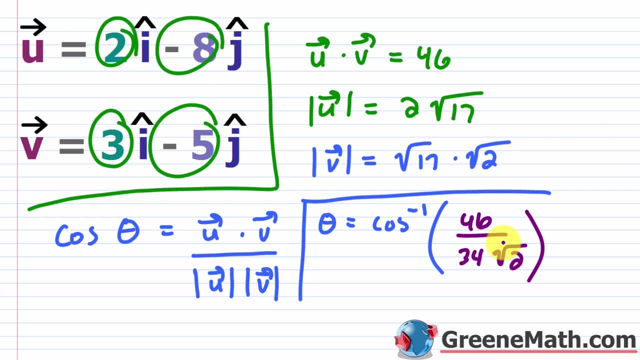 but for the purposes of punching it into a calculator. who cares right? It's just going to work either way. So again, if you're having problems with this, wrap this in some parentheses. And if I punch this into my calculator, I get a theta that's approximately 16.93 degrees. 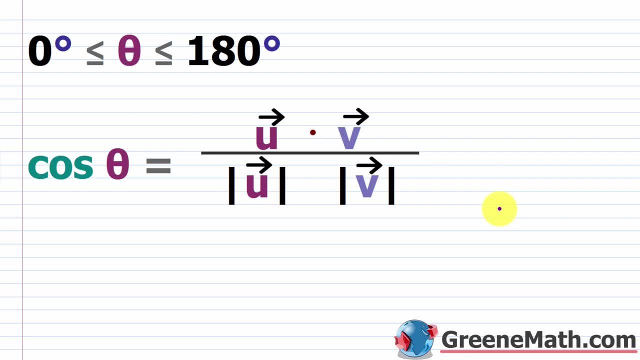 All right. So before we wrap up the lesson, let's talk about the concept of orthogonal vectors. And this is just a fancy word to say that you have perpendicular vectors. Okay, So they're going to meet at a right angle. So when the dot product for two non-zero vectors- again u and v- is zero, then what's going to happen? 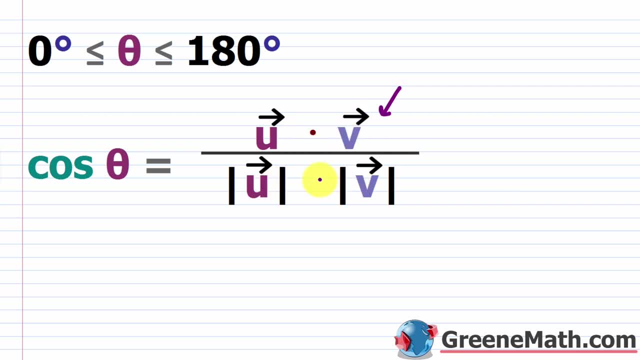 is, the top part of this formula here is zero, And because you have non-zero vectors down here, the bottom part, or the denominator, will not be zero. So zero divided by something that's not zero is always going to be zero. Okay, So then you could say: the cosine of theta is going to be equal to: 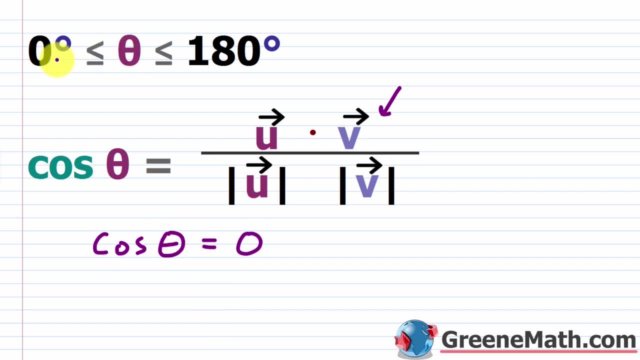 zero. And where does this happen? Again, if theta is greater than or equal to zero degrees and less than or equal to 180 degrees, well, it must be true that theta is equal to 90 degrees. So the angle between these two vectors, 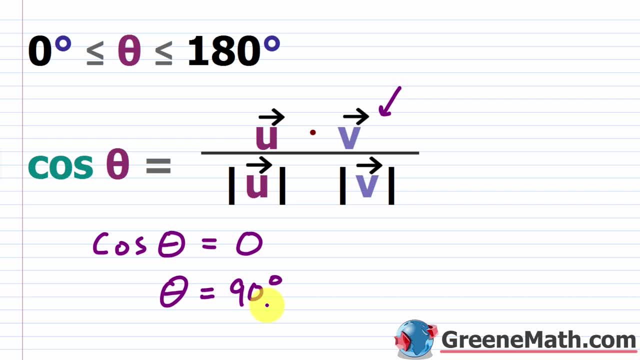 u and v is going to be 90 degrees, meaning these two guys are perpendicular vectors or, in the language of vectors, we say they're orthogonal vectors. Okay, So all you need to do if you want to check to see if you have these orthogonal vectors, is just do the dot product. 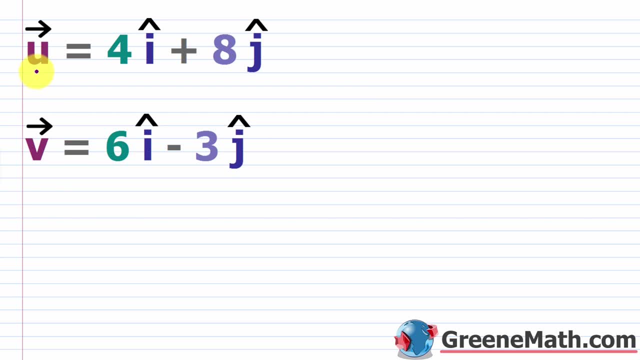 and see if it's zero. That's all you want to do. So, to start out this problem, I have this vector u, which is going to be four times the unit vector i, plus eight times the unit vector u, plus three times the unit vector j, And then I have this vector v, which is going to be six times. 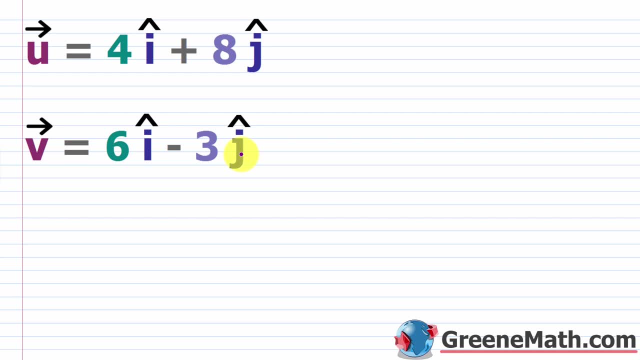 the unit vector i minus three times the unit vector j. Okay, So if I wanted to find out if these two vectors were perpendicular or, again, if they were orthogonal vectors, I could just find the dot product and see if it's zero. Okay, So in other words, with your formula, cosine of theta is equal. 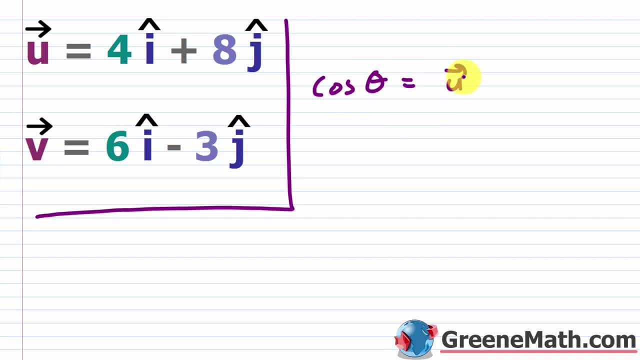 to: you've got your dot product okay, which is the dot product of u and v. So u dot v, okay, over the magnitude of this vector u times the magnitude of this vector v. Okay, So we know this formula at this point. Again, if this top part ends up being zero, 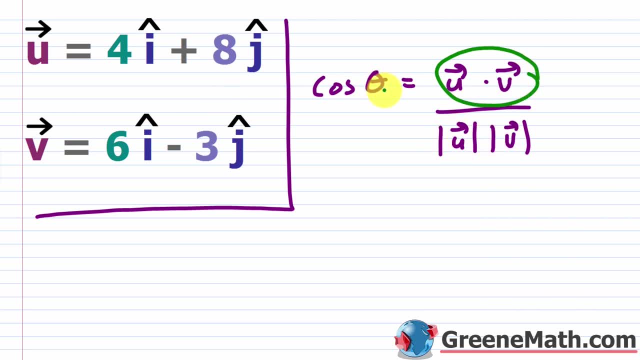 and these guys down here aren't zero- which they won't be- well then the cosine of theta will be equal to zero and theta is 90 degrees right, So these guys can be perpendicular. So the dot product here- okay, we do u- dot v is equal to four times six, is 24.. And then plus eight times negative three. 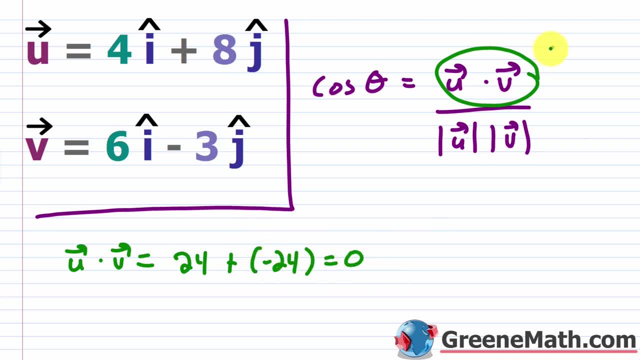 is negative 24.. So of course this is zero, right. So again, this top part would be zero. the bottom part wouldn't be zero. you can go through and find the magnitudes multiplied together and you'll see in the end, So zero divided by something that's not zero, you just get zero, right. So the cosine? 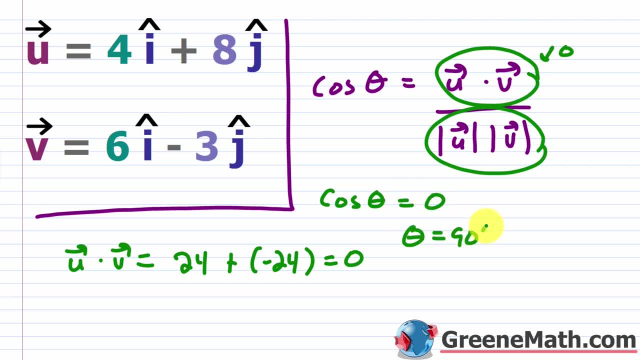 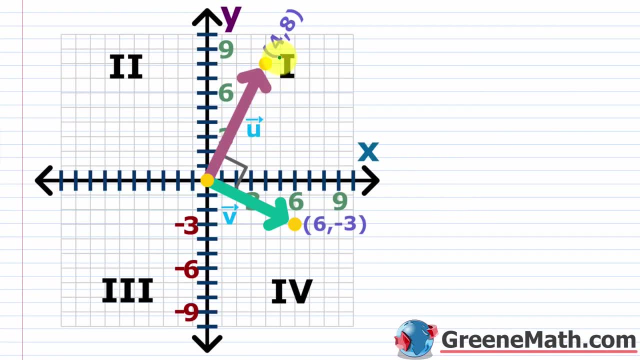 of theta is going to be zero, So theta equals 90 degrees. And, of course, we have perpendicular vectors. If you want to see this, your vector u okay, which we have right here. the terminal point is at four comma eight, right, Because again, this vector u was set up as four. i. 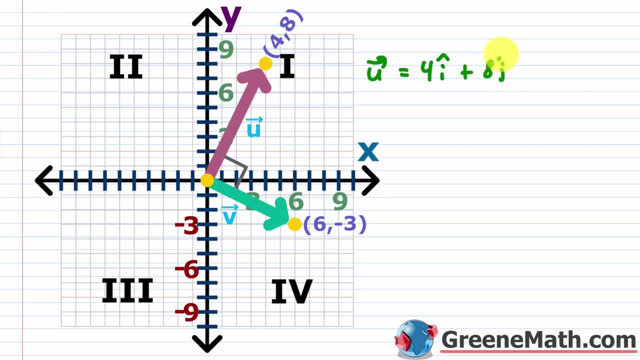 okay, that unit vector, plus we had eight j. that unit vector. okay. And then for the vector v, the terminal point was at six comma negative three. here's the vector v, again, you're going to have this 6 times the unit vector i, plus you're going. 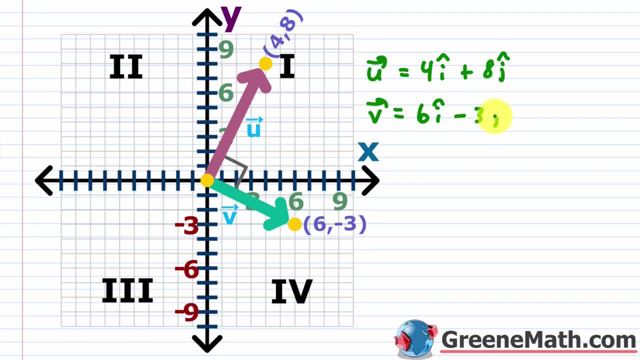 to have this negative 3, or might as well just write minus 3 times the unit vector j. okay, so this is how we set this up. so this guy has a terminal point at 6 comma negative 3. this guy has a terminal point at 4 comma 8. you can see this graphically that they're going to meet at a 90. 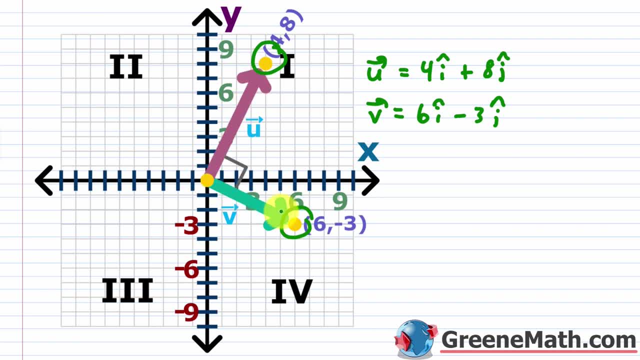 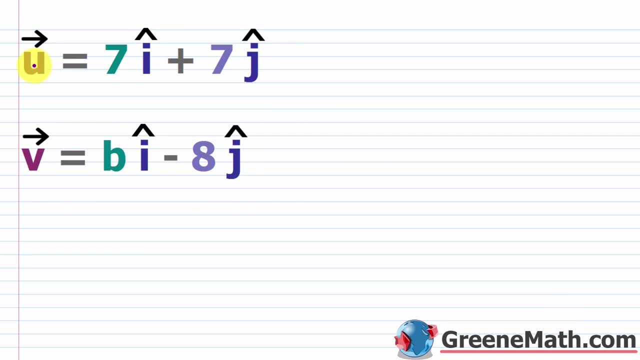 degree angle and therefore, by definition, these guys are perpendicular, or you could say they're orthogonal vectors. all right, as a last example, what if you had something like this: so we have our vector u and it's equal to: we have 7 times the unit vector i plus 7 times the unit vector j. 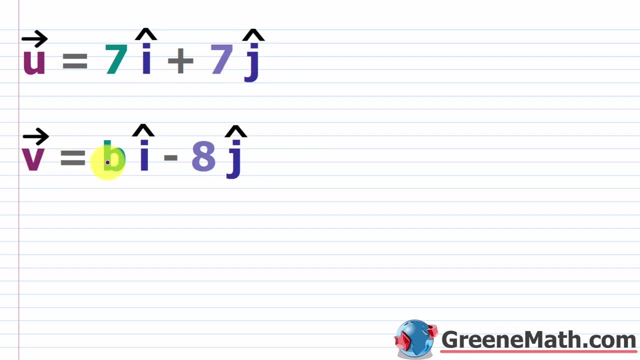 then we have this vector v and it has b. okay, some unknown times the unit vector i minus 8 times the unit vector j. how can i find a value for b such that the two vectors u and v would be orthogonal, or you could say perpendicular vectors? well, all you'd want to do is just set up your little dot. 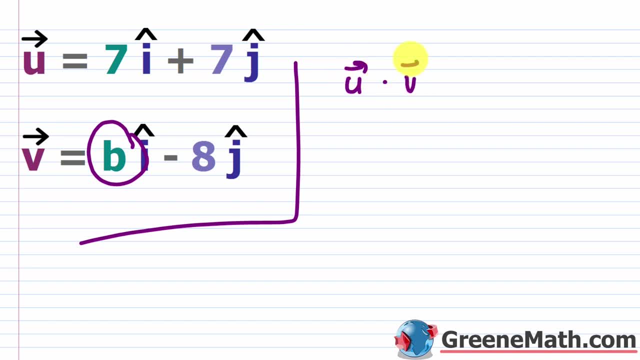 product. okay, so the dot product of u and v is going to be what? 7 times b, so 7 times u, and v is going to be 7 times u and v is going to be 7 times u and v is going to be 7 times v, and then plus you're going to have 7 times negative 8, which is negative 56, so you 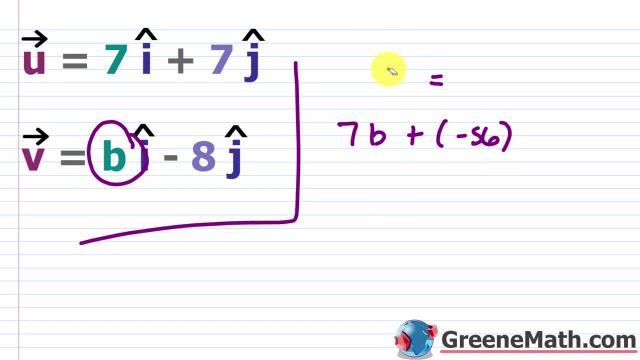 really need this guy right here. you can just substitute this with a value here. you really want this to be 0? let me just do this down here. so you really want this to be 0, so that those guys can be orthogonal vectors, right? so i'm just going to solve this equation for b and to do that i'm 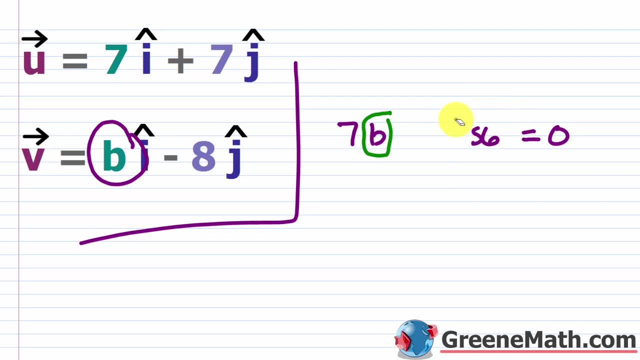 going to add. let's just go ahead and write this as negative 56 or minus 56. so i'm just going to add 56 to both sides of the equation. okay, so this would be gone. let me just write this as: 7b is equal to 56. obviously. this is very simple. divide both sides by 7. you'll find that b is. 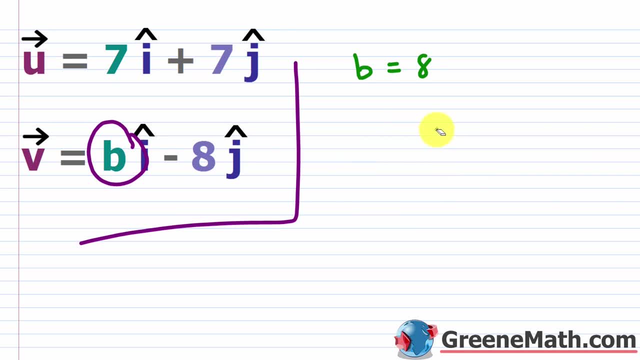 equal to 8. okay, very, very easy to do these. and again, if you plugged in an 8 there, well then, the dot product from your vector u and your vector v, so u dot v, would be what? 7 times 8 would be 56, and then plus 7 times negative 8 would be negative 56, so the dot product would be 0 and in this case, 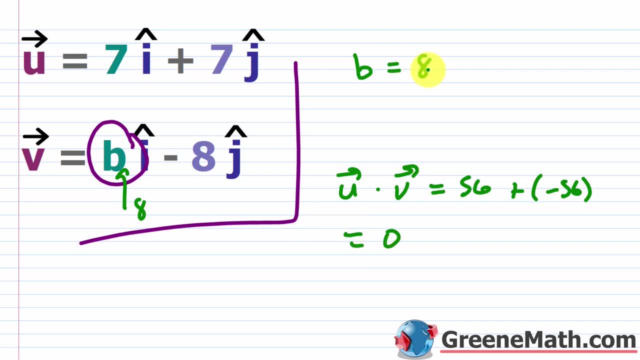 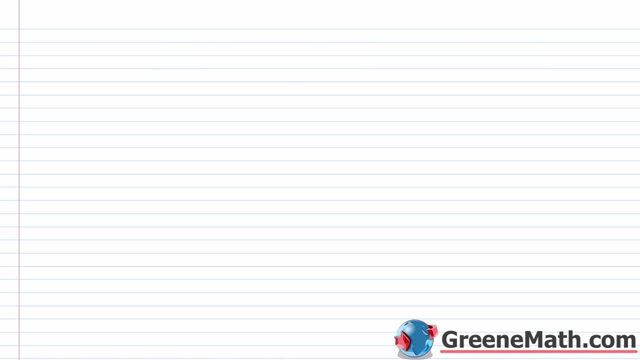 if b is 8, well, you would have perpendicular vectors or again, orthogonal vectors, vectors. in this lesson we want a review of complex numbers, all right, so i want to start out by talking about the imaginary unit i again. so we say i is equal to the square root of negative 1 and this: 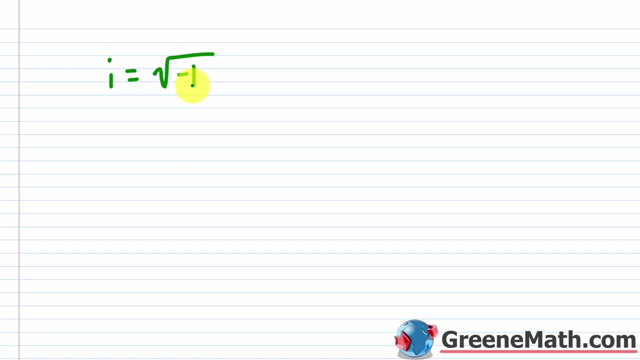 is used to allow us to simplify when we have the square root of a negative number. so, for example, if i had the square root of, let's say, negative 4, using the product rule for radicals, i could write this as the square root of negative 1 times the square root of 4. okay, i know that the square root 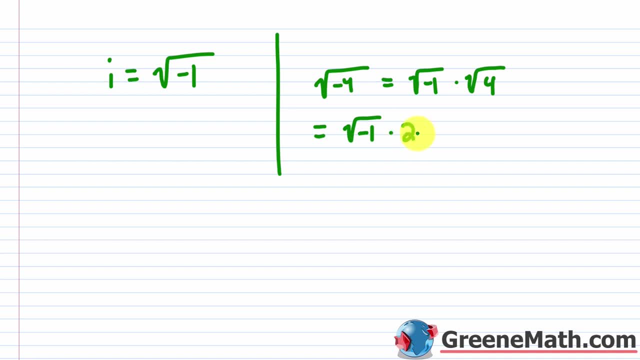 of 4 is 2, so let me just go ahead and write this as the square root of negative 1 times the square root of 4. let's go ahead and put the square root of negative 1 times 2, like this, and then i can replace the. 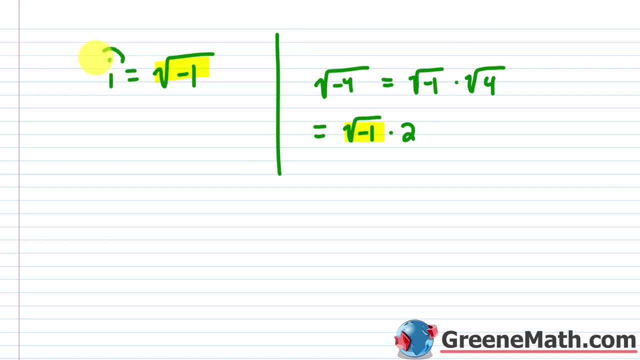 square root of negative 1. okay, since those guys match up with this, i here. okay, so this can go right there. so this is i times 2, or just write 2i, okay. so that's a way to simplify the square root of a negative number. now also, let me erase all this. we can square both sides and come up with 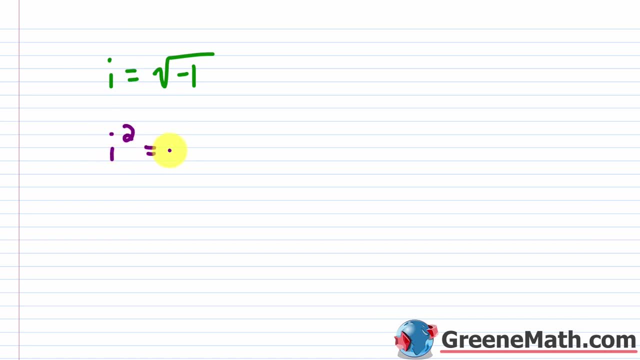 another definition. we could say that i squared is equal to negative 1. we're going to use this all the time. okay, now, using the square root of negative 1 times the square root of negative 1, we're going to add another dimension to this square root of negative 1 times 2, and that's. 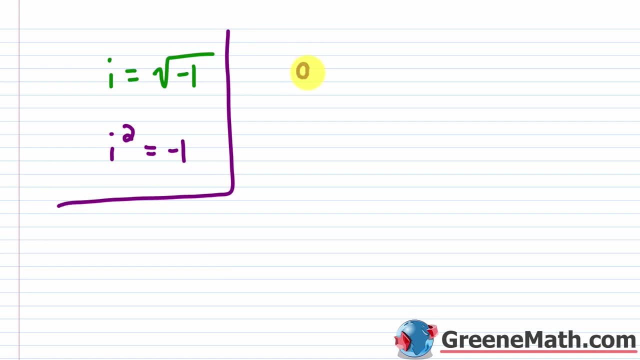 going to be negative 1 against negative 2, and this one isn't a square root of negative 1. so the square root of negative 1, it's negative 1, square root of negative 1. goddess andεις, okay, at the last step, we're going to add a new dimension right now into the square of. 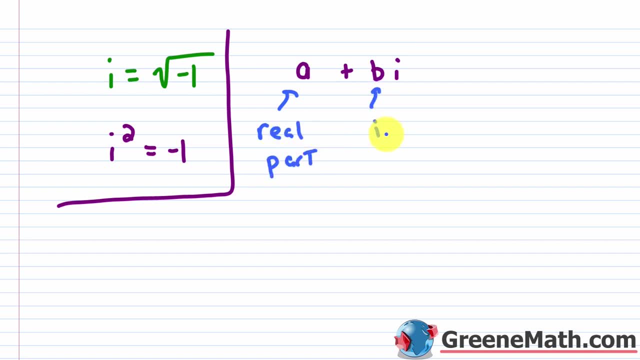 negative: 1. okay. okay now, depending on your scale, where you YU and this�, you can see that we're going to start off by specifying the quorum of the order. we're going to be bi the imaginary part. just get with your book or your teacher in terms of what they want to do if 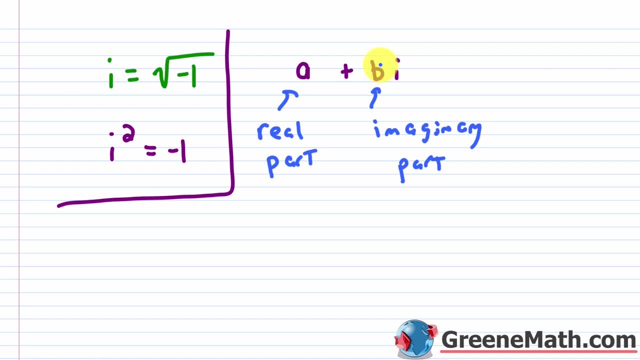 you get this for vocabulary now, in terms of complex numbers, we don't often think about it this way, but if you just had the number, let's say three, well, three is a complex number. okay, three is a complex number because i could always say three plus zero i. it's kind of like when you think about three as 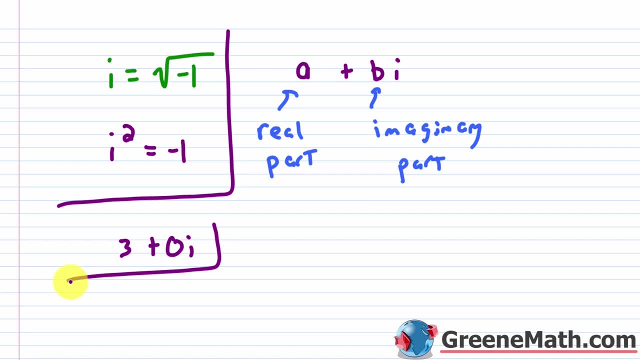 being a natural number, right, it's a whole number, and then it's an integer, and then it's a rational number. and the way you show it's a rational number is you go: okay, well, three is equal to three over one, right, those are the same. so this is, by definition, a rational number, so it's the same. 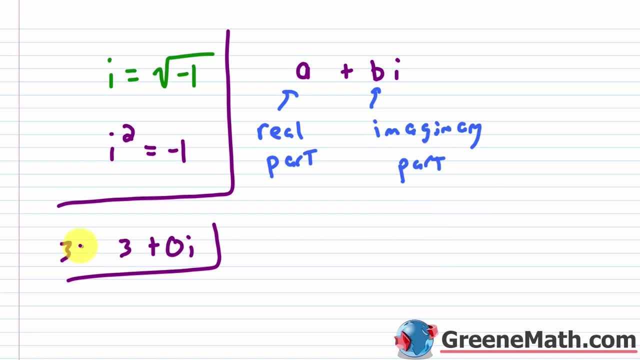 kind of trick here where we just say, okay, well, three is really equal to three plus zero i, because this is just zero, and three plus zero zero is still three. okay, so this tells me that any real number that i'm working with is also a complex number. so the real numbers are a subset, okay, of 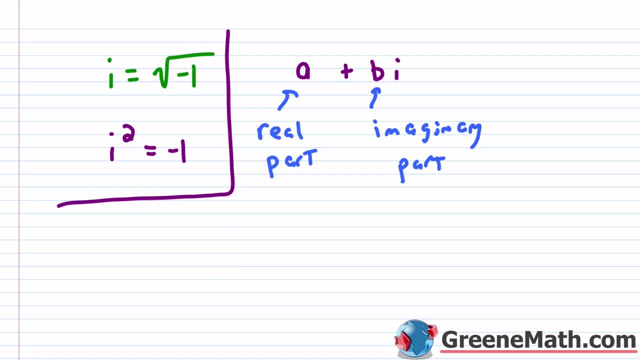 the complex numbers. and if you have a complex number, okay, like let's say you have a complex number, let's say four plus two i. this is called a non-real complex number. that's how you can differentiate between the two. also, you can have something that's called a pure imaginary number. 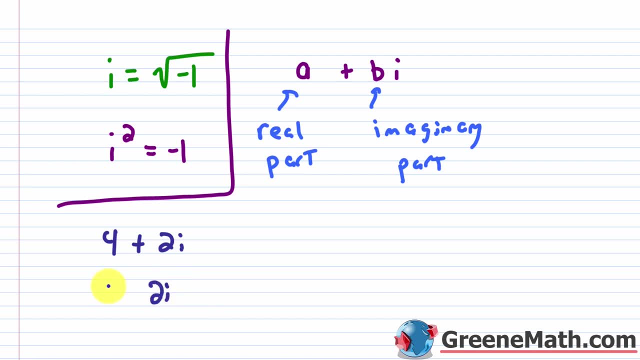 let's say you just had the two i part. okay, so this you could write as zero plus two i, which is just two i. this is also a non-real, complex number, but a lot of books will call this a pure imaginary number. okay, let's go ahead and look at some examples. we're just going to fly through these. 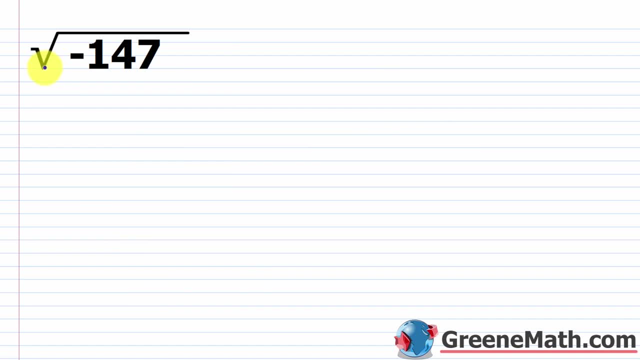 again, this is just stuff we've already seen here, so let's go ahead and look at some examples. if you wanted to simplify the square root of something like negative 147, you would use your product rule for radicals. i would just put this negative one here times you would try to factor. 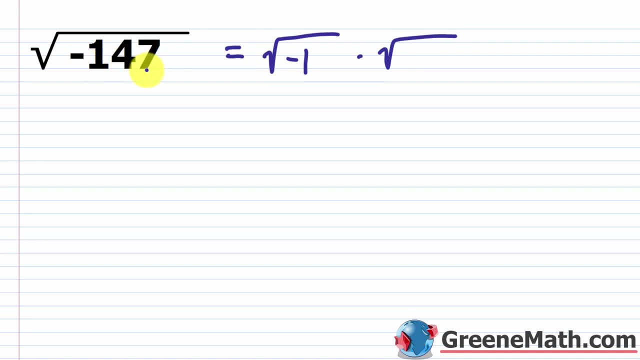 this. well, one plus four is five. five plus seven is going to be 12. i know that 12 is divisible by three, so 147 will be divisible by three, and if i divide 147 by three, i'm going to get 49, so i can. 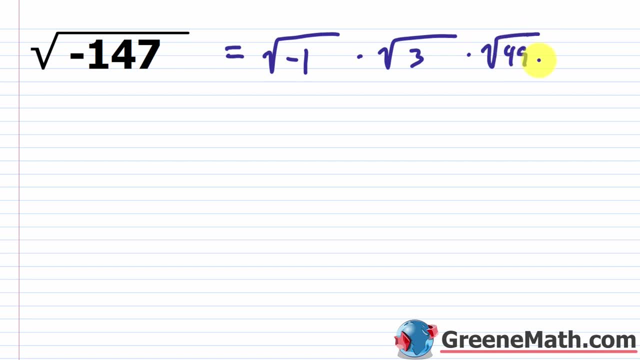 put a three here and i can get a square root of 49 here. okay, and this guy is a perfect square, so the square root of 49 is seven. so what i can do here is say that this is equal to square root of negative one times square root of three. okay, then times seven. now this guy right here. i can always. 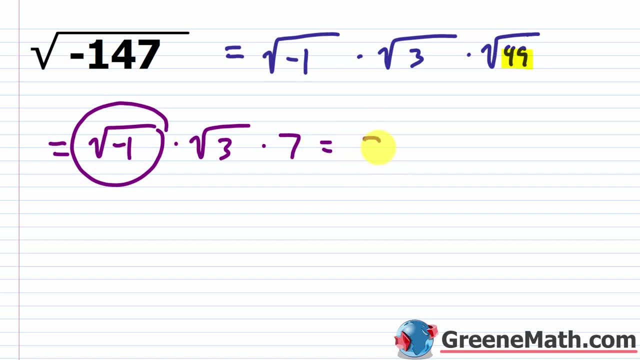 replace with i. so really, i'll end up with just saying that i have seven. i okay, times the square root of three. so this would be our simplified answer for this square root of negative 147: again seven i times the square root of three. all right, another similar problem. we have the square. 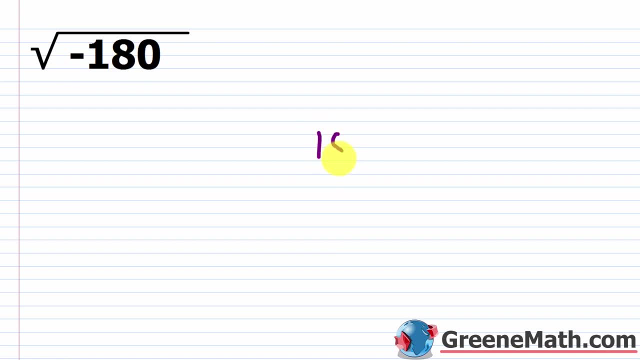 root of negative 180. so for this guy, if i think about 180, i'm going to put this square root of 180. i would factor this: so one plus eight is nine, so i know it's divisible by nine. so let me go ahead and put nine there and this would be 20, right? so nine is three times three. those are prime 20 is. 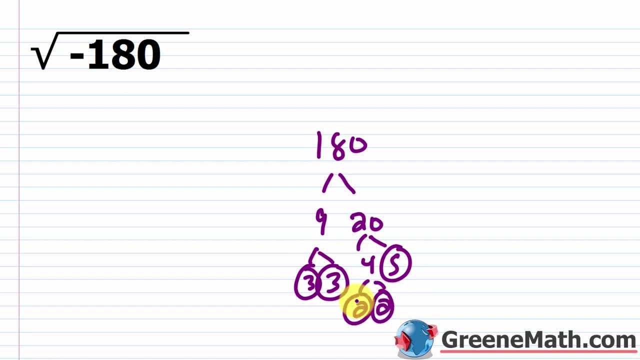 four times five. four is two times two, so what i'd want to do, since nine is a perfect square, and so is four, multiply those together, you have 36. so basically, you'd want to write this as square root of negative one times square root of 36 times square root of five. okay, so that's going to allow. 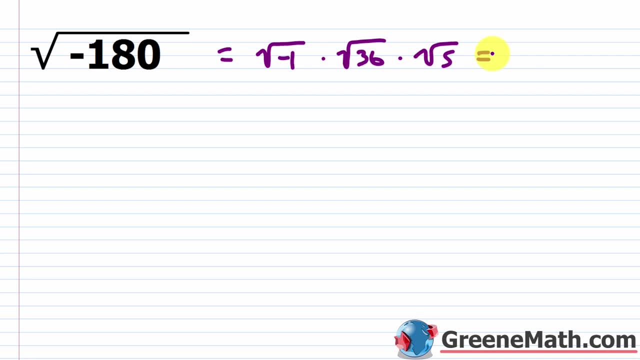 you to simplify, and basically square root of 36 is six and square root of negative one is i. so i'm just going to put that we have i times six, or i should really rearrange this and put six i, and then just times the square root of five. okay, so simplifying. 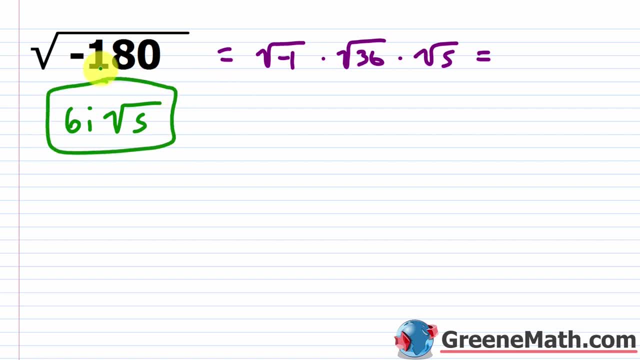 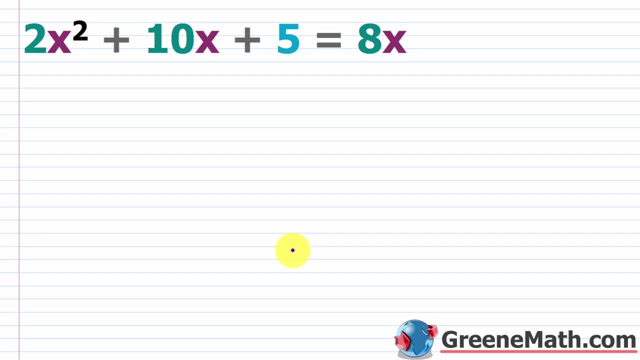 these types of problems very, very simple. this is our answer again: the square root of negative 180. this is going to simplify to six. i times the square root of five, all right, so, additionally, you will see complex numbers when you work with equations such as a quadratic equation. we know. 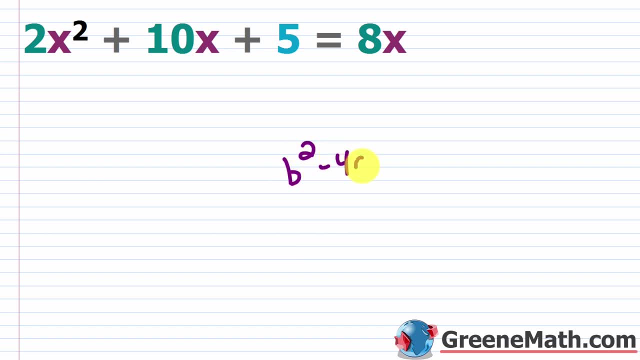 that if the discriminant, that b, squared minus four, ac part, if that's less than zero, you're going to get complex solutions, okay, so we're going to see that here. so i'm just going to solve this. i'm going to use the quadratic formula. if you want to complete the square, you can do that on your. 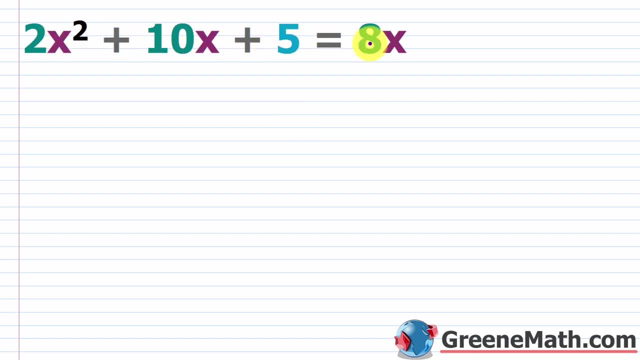 own. so i have 2x squared plus 10x. plus 5 equals 8x. i'm going to subtract 8x away from each side to put this in standard form. so this is going to cancel over here and be zero. so i'm going to have: 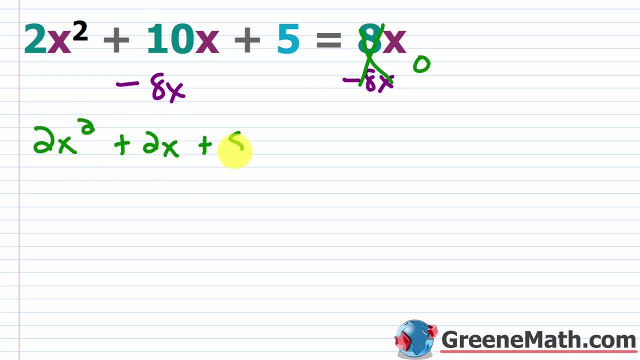 2x squared plus 2x plus 5 equals zero and basically i'm going to record the values for a, b and c. okay, coefficient for x squared. so this guy right here. so that's a, two, and then what's b? it's going to be. 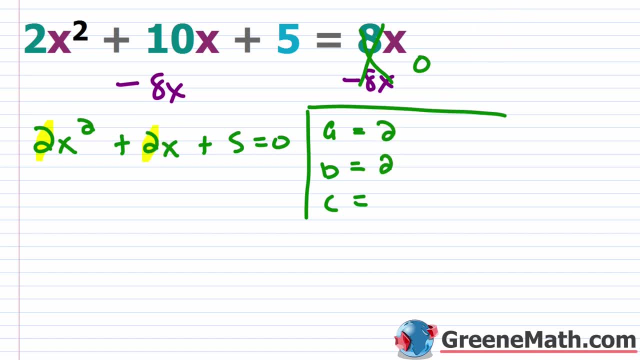 the coefficient for x to the first power. so that's also a, two, and then what's c? that's going to be your constant term. so in this case, that's five. okay, and then you're going to plug in. so x equals- remember this is negative- b plus or minus the square root of b, squared minus 4ac, all over 2a. 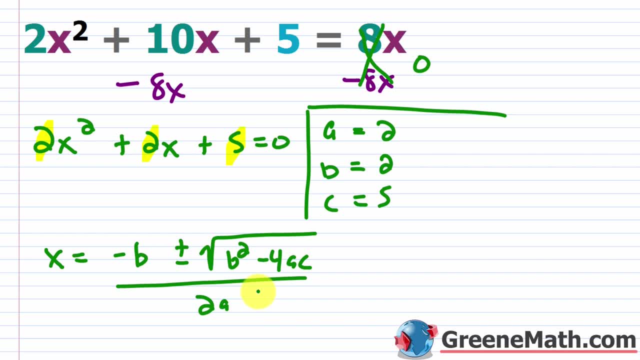 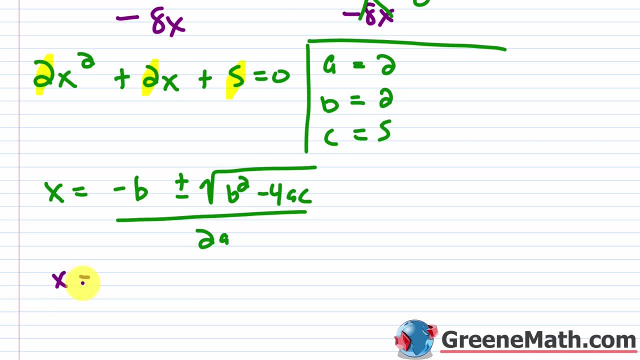 okay, this is something i've memorized throughout the years. if you don't have this committed to memory, it's okay, something you can really look up quickly. okay, so i'm just going to scroll down a bit and i'm going to plug in. so x is equal to the negative of 2, plus or minus the square root of. 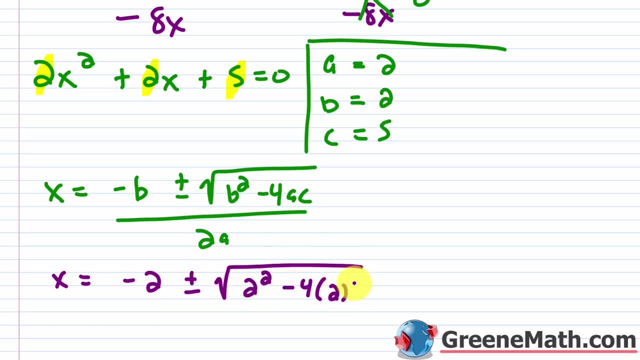 you're going to have 2 squared minus 4 times 2 times 5, and all i'm doing is i'm just plugging in. okay, this is over 2 times 2, so i plugged in for b, a and c and that's where we got this from now. 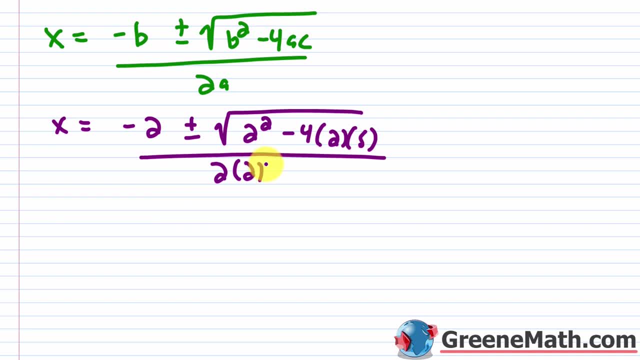 let's just go ahead and solve this real quick. it's just a matter of punching this into your calculator. so x is equal to negative 2 plus or minus the square root of you have 2 squared, which is 4 minus 4 times 2 is 8. 8 times 5 is 40. go ahead and do 4 minus 40. that's going to be negative 36. 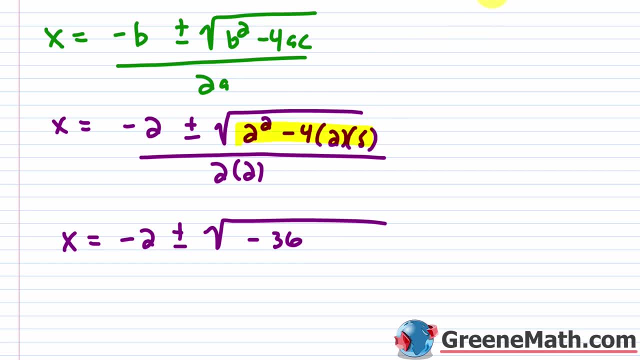 and you can see, because this part right here ends up being negative, you're going to have these complex solutions. okay, then this is over the 4, because 2 times 2 is 4 and then the square root of negative 36. you can say that is 6i. right, square root of 36 is 6 and then square root of negative. 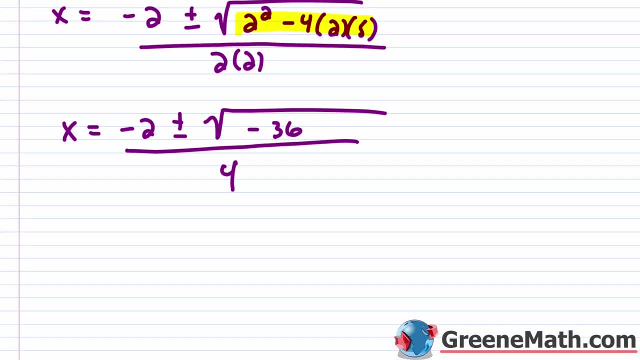 1 is i. let's come down here a little bit and let's go ahead and say that x is equal to negative 2 minus i'll put 6i over 4. now we can factor out a 2, okay, and make this a little bit better. so let's. 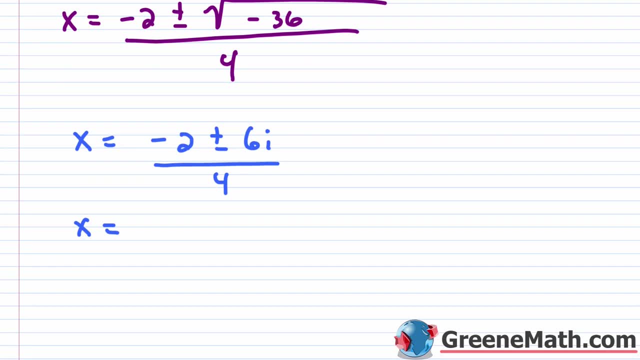 go ahead and say x is equal to. let me pull this down here a little bit. i'll factor out my 2. i'll have negative 1 plus or minus 3i. okay, then, over 4. i'm going to cancel this with this and put a 2. 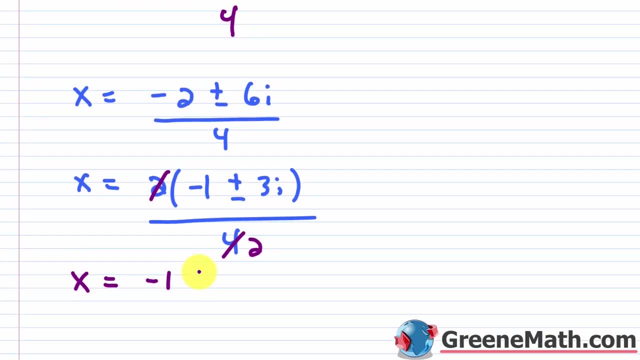 here. so we'll say x is equal to. you have negative 1 plus or minus 3i over your 2. now, if you want to write this in standard form for the complex number, you're going to have negative 1 plus or minus 3i. 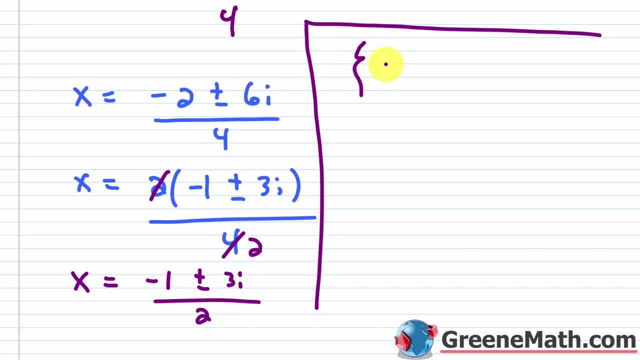 over 4, then you can put this: go ahead and do solution set notation. i'll put negative one half, okay, like this, and then i'll go plus or minus. we'll do three halves and then times: i like this, okay. so that's your solution set notation. maybe i can make those brackets a little bit better. 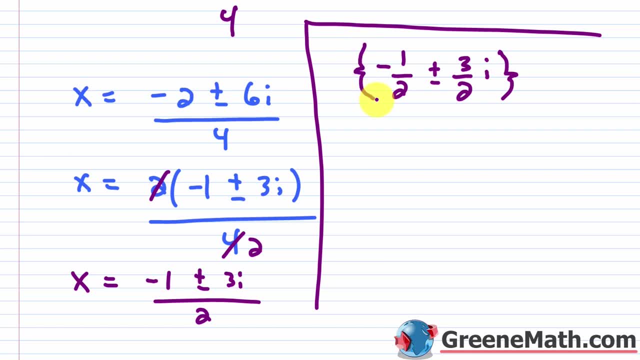 let me try to make this one a little bit better, like that, okay, and of course this is two different solutions. right, you have negative one half plus three halves times i, and then you have negative one half minus three halves times i. all right, let's start working on some. 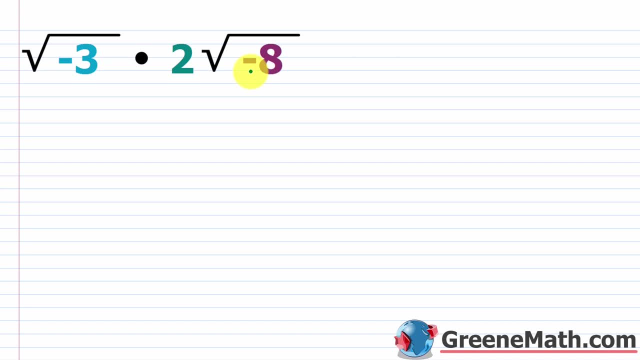 operations with complex numbers now. so the first thing i'm going to do here is a simple multiplication problem. i'm doing this to draw your attention to a common mistake. so we know, with the product rule for radicals, something like square root of a times square root of b. 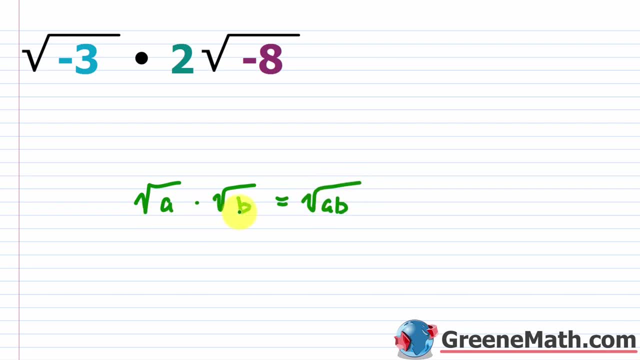 this equals the square root of ab. this only works when they're both not negative. okay, so if you try to do this here, you're going to end up with the wrong answer. so what you have to do when you have negatives involved like this, you have to convert them over. okay, simplify first and then go through. 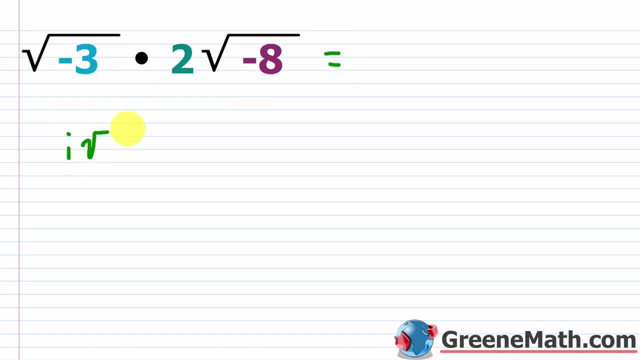 a multiply. so what i would do here is i would say this is: i times the square root of three and times for this one. let me go ahead and write this out, so we'll have two times. i'm going to put the square root of negative one times the square root of four times the square. 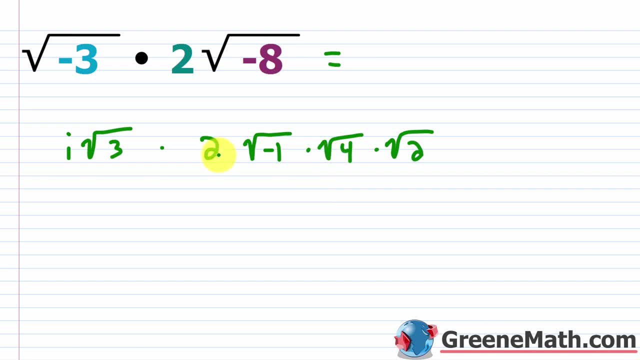 root of two. okay, just so you can see what i'm doing. square root of four is two, so two times two is four, okay, and then basically you would have square root of negative one, which is i, so this becomes four. i times the square root of two. okay, so from here now, if you multiply, you see that you. 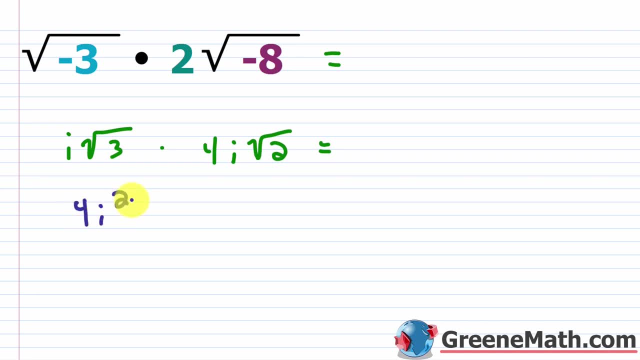 have one or two. i times the square root of four plus or log produto of g of an times the normal prime. the table is equal toượng square root of three times the square root of two. okay, and if i just use this straight from here, it's actually going to do this and i really 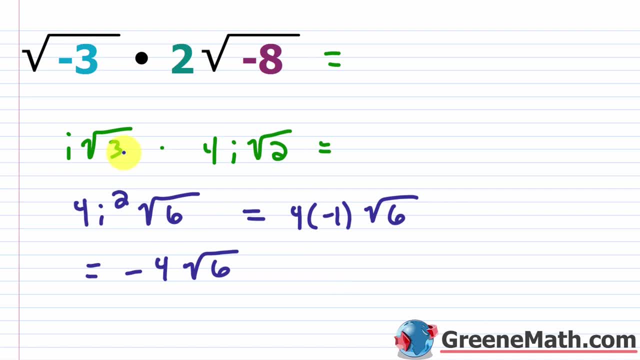 want to hè. v equals negative, one by negative of d. the problem is, if you write in the minus à, go to the square root of one which is negative, 1, which is negative, and then i'm going to have 4i, which is one second important things, right? so that's what we've done here. so if i use the square, 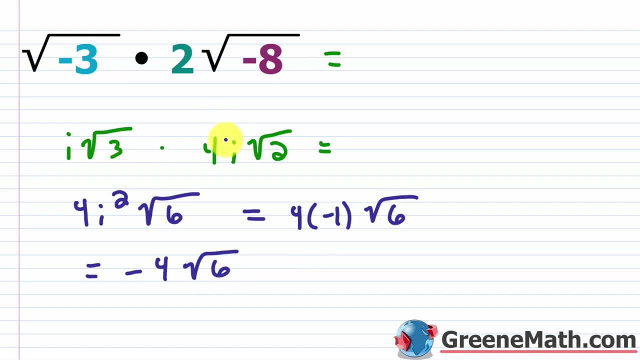 root of 4i, which is negative. i times the square root of 2, where it's negative, c, which is negative, 1.. four times negative, 1 times the square root of four, which is gonna be what that means. So you want to make sure you convert these over. simplify them first before you multiply. 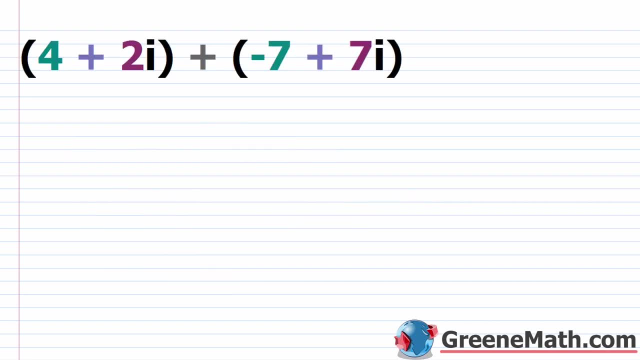 Okay, let's look at some addition of complex numbers. Really really easy topic To add two complex numbers. so, for example, if I have A plus B I and then I add this to, let's say, C plus D I, okay, this is what. 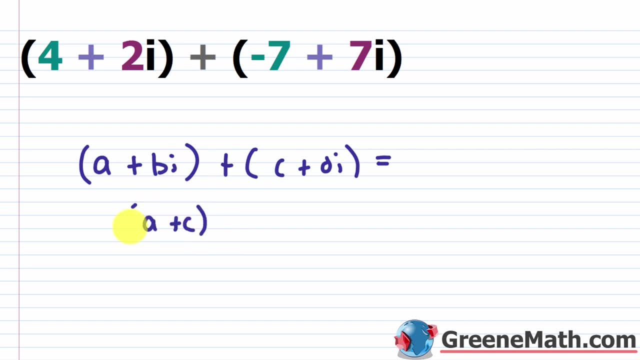 Add the real parts, so A plus C, okay, and then plus, you're going to add the imaginary parts, so we'll say B plus D, okay, and this is multiplied by I. That's all it is. If you were subtracting, okay. so if this was a minus, then this would become a minus. 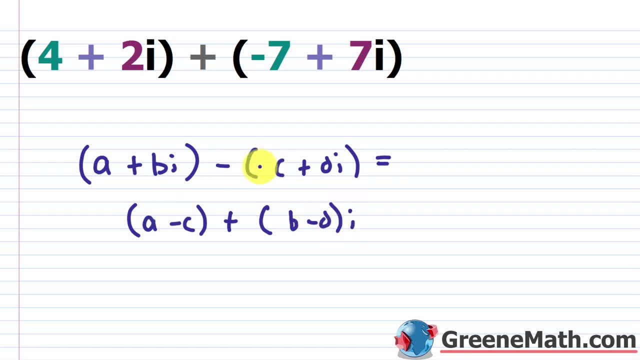 and this would become a minus. and that's basically it. Now, when you subtract things away, remember you can do addition of the opposite, so you could always go plus and then minus and then minus, like this. okay, so if you want, 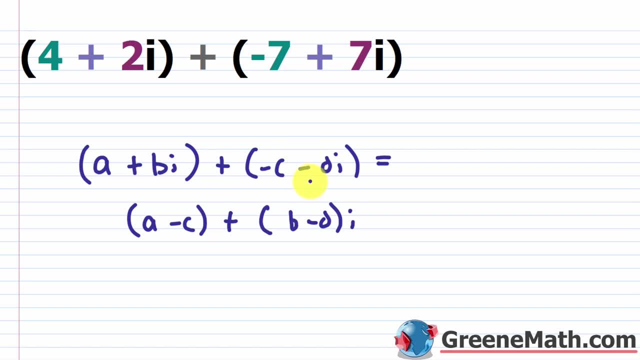 to do that. you can do that. Either way, your answer is going to be the same, okay? so let's go ahead and get rid of this and let's work on this problem here. so we have four plus two. I plus we have negative. 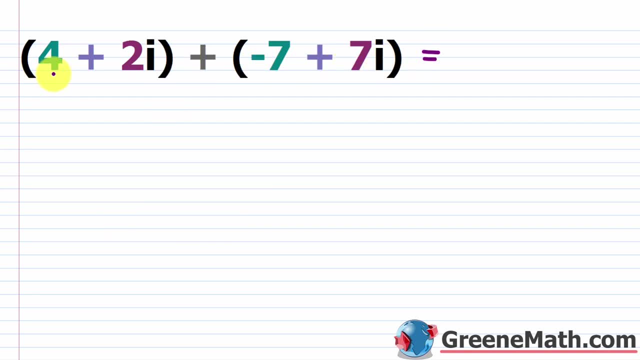 seven plus seven, I okay. so what do we do? We add the real part, So four plus negative seven. let me show this. so four plus negative seven, okay, and let me put a parenthesis there. and then, plus you add the imaginary parts, so two plus seven. 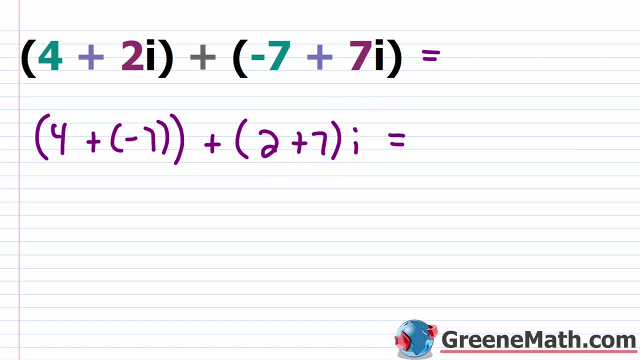 so two plus seven. okay, then times I out here, and let's go ahead and simplify this. so four plus negative seven is negative three, and then plus two plus seven is nine, and then times the imaginary unit I. So this is your answer here, okay, and it's in standard form. so negative three plus nine. 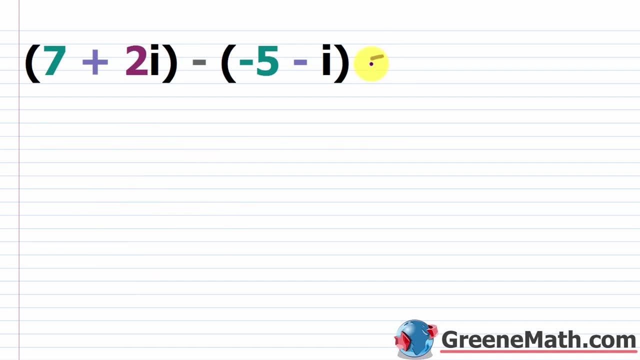 I All right for the next problem. let's do a subtraction so you can do this as addition of the opposite, If you want. so I'm just going to go ahead and say this is seven plus two. I okay, I'm. 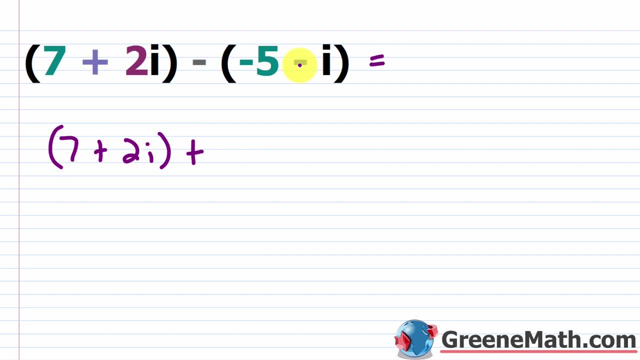 going to say plus and I'm going to change the sign of everything inside. It's just like if I put a plus here and a negative one outside and distributed this to each term. okay, that's all I'm doing. okay, I think it makes it a little bit simpler. 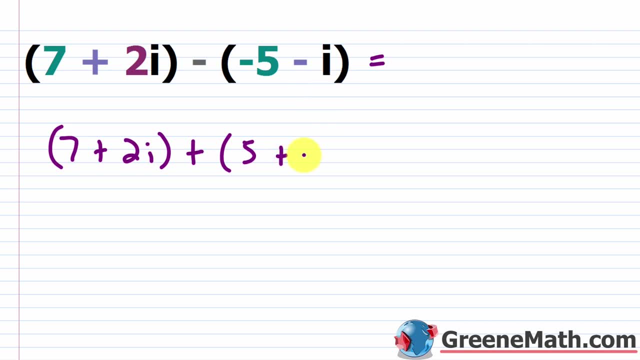 so I'm going to change this to positive five and I'm going to change this to positive. I'm going to write a one and then times. I Remember, if something's hanging out by itself like X, you can put a one in front as the. 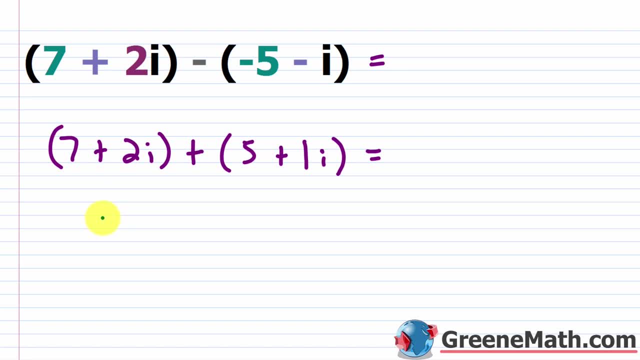 coefficient, okay, so now I can just add: so this will be seven plus five, Okay, and then plus, you're going to have two plus one, okay, and then times I. so this gives me 12 plus three I. as a result, and again, if you want to do this with subtraction, 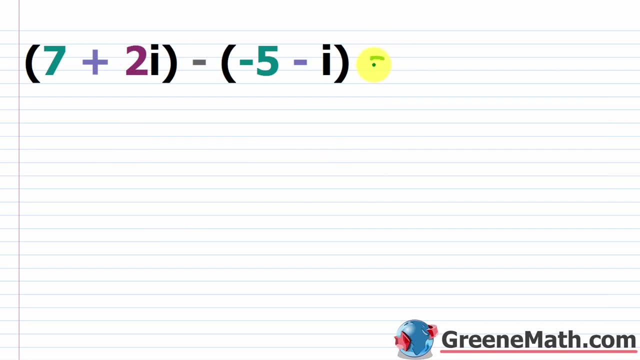 you can. It's going to look a little bit different. so what you can also do is you can say that you have seven minus. in this case, this is a negative five, so be very careful, okay. and then you have plus. you're going to have two minus. this is a negative one, so again, 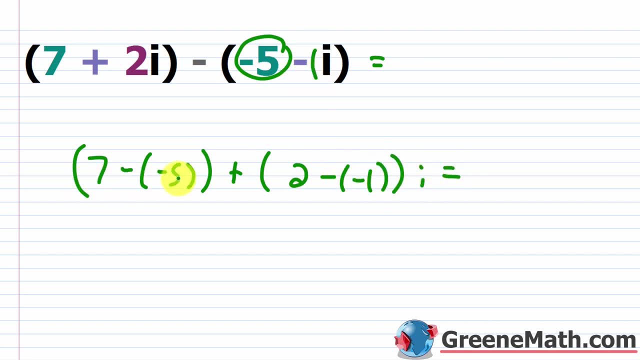 be careful, okay. and then times I here Seven minus a negative five is 12, and then plus two minus a negative one is three. and then times I. So same answer either way. I think it's more straightforward if you do. addition of the. 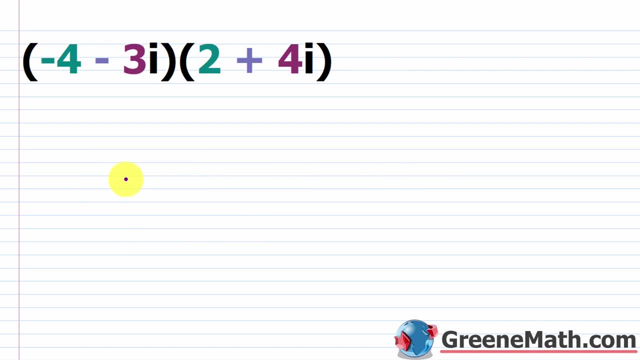 opposite. Let's look at some multiplication Again. with these type of problems, you can generally use FOIL- okay, and sometimes you'll get longer ones, just depending on the situation. but just pretend like you're multiplying polynomials, okay. 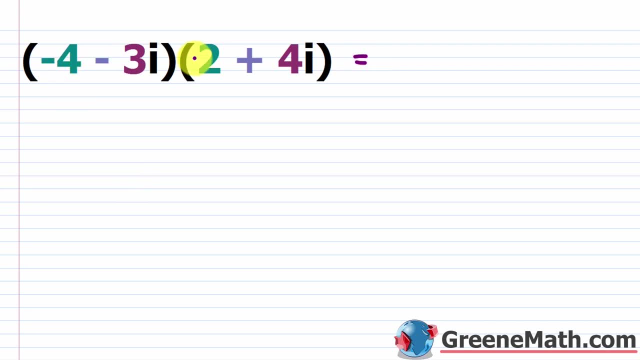 So I'm going to use FOIL here. so I'm going to do the first terms: negative four times two is going to be negative eight. and then my outer: negative four times four I, It would be minus 16 I. My inner, I would do negative three I times two, that's minus six I. and then my last: 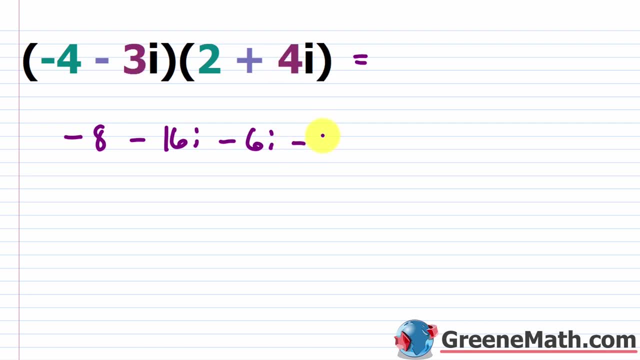 I would do negative three I times four I, which would be negative 12. I squared okay, So I squared is negative one, so let's go ahead and replace that. So I'm going to have negative eight, and then I'll go ahead and move this down and say minus. 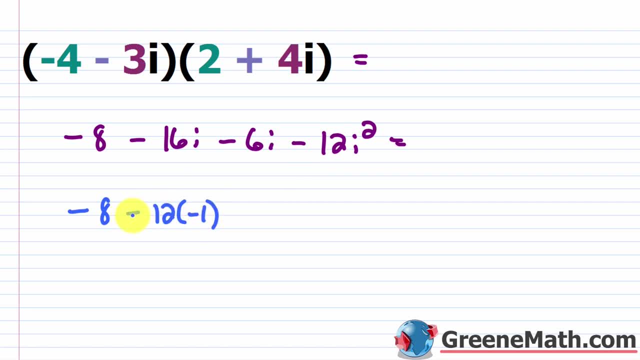 12 times negative one. Well, negative times negative is positive. so I might as well just say: this is plus 12, okay. and then I have this: it would be minus 16 I, So I can say: that's minus 22 I, so negative eight plus 12 is four. and then we'll say: 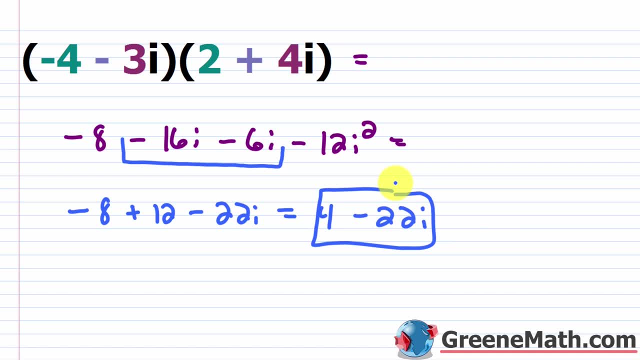 minus my 22, I okay. so that's going to be my answer there and I boxed that off a little bit too closely. So four minus 22, I All right. so we should know at this point about conjugates. If you have complex conjugates, the formula is a little bit different. 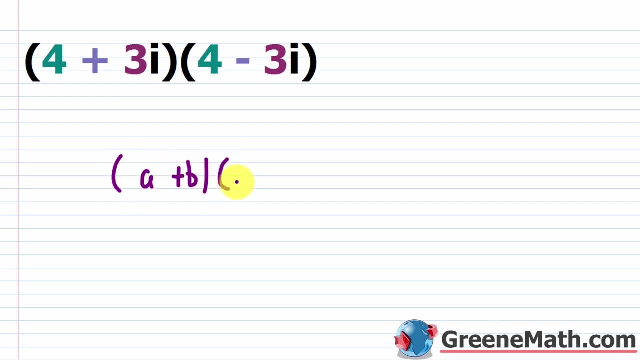 So if we have something like A plus B, times A minus B, we know this is A squared minus B squared. okay, As an example, let's say I have something. I have something like X minus two. okay, then I have X, let's say plus two. 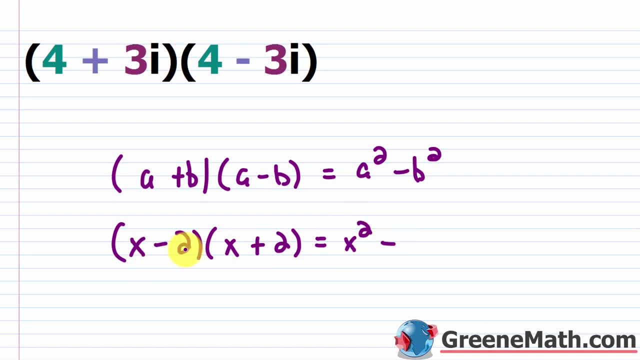 I know this is X, squared, which is the first guy, minus two squared, which is the second guy, which is four. okay, I don't need to FOIL this out. That's the quicker way to do it, but if I'm dealing with complex conjugates, the sign 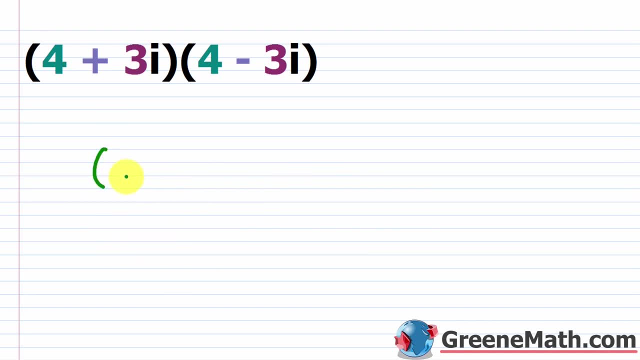 is going to change. It's not going to be minus, It's going to be plus. So, for example, if I have A plus B, I times A minus B, I, what happens is A times A is A squared. The outer and the inner are going to cancel. 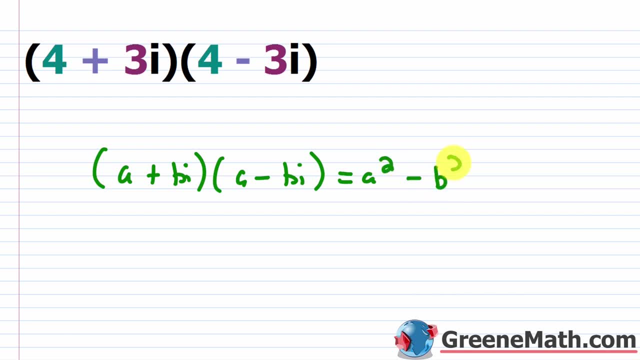 And then the last you have your minus B squared times I squared. Well, this I squared here is negative one and that's what's changing the sign. So you end up with A squared plus B squared. okay, So if I look at this pattern here, I have four plus three. I times four minus three, I. 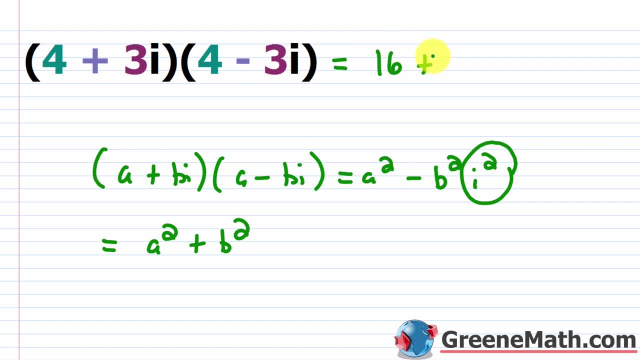 I can just say: okay, the first guy squared, four squared is 16, plus this three guy here, the second guy, just the B part, just the imaginary part. So the three guy squared, which is nine, so that's 25.. 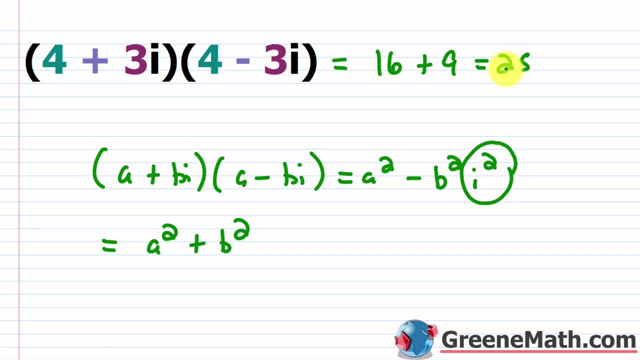 Okay, This is always going to be just a number, So in this case it's just going to be 25.. Okay Again, if you wanted to go through this the long way we can, just for the sake of completeness. 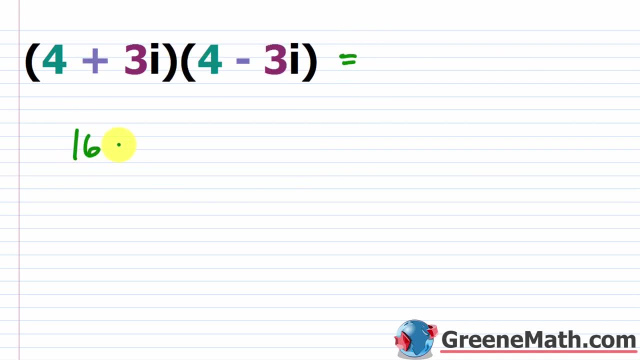 we would do first times first. So four times four is 16.. And then the outer would be negative 12 I, The inner would be positive 12 I. So you see those guys are still going to cancel. Then for the last, you have three I times negative three I. 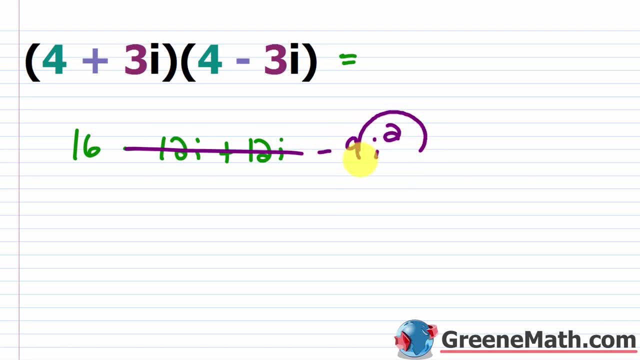 So that's minus nine I squared. And again, the I squared here is going to change the sign And I circled that a little bit too widely, but basically this is what This is: 16, you might as well say minus your nine times negative one. 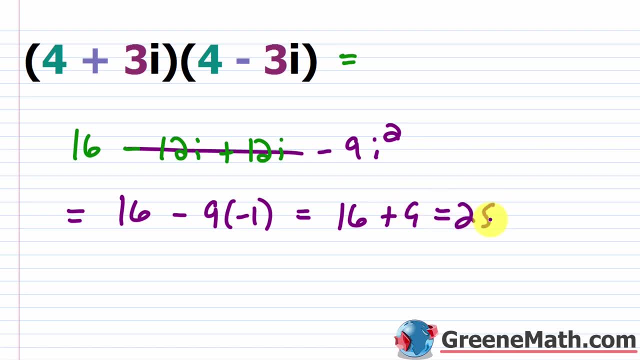 which is 16, basically, plus nine, which again is 25.. Okay, Let's talk about dividing complex numbers now. So we know that if the imaginary unit I is in the denominator, since I technically is the square root of negative one, it represents a radical. 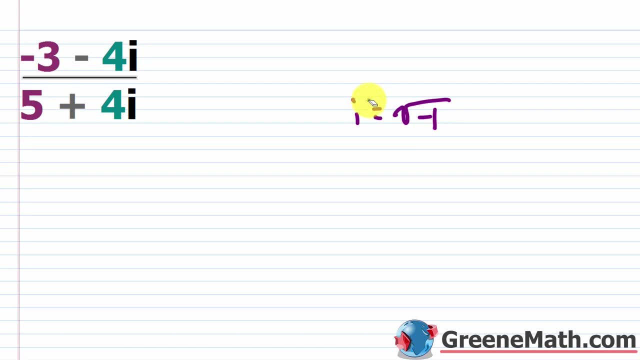 It needs to be rationalized, right? So we want to rationalize the denominator when we see this situation. So if I have something like negative three minus four I, over five plus four I, what can I do? Remember we just talked about multiplying by the complex conjugate. 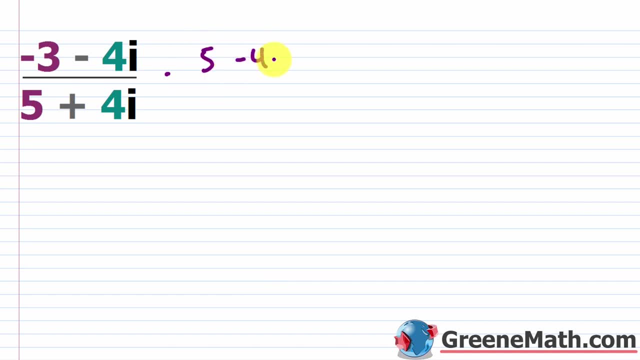 If I multiply this by five minus four, I over five minus four, I. what's going to happen is in the denominator. here I'm going to have a real number now. Okay, We don't care what happens in the numerator, We're trying to get the radicals out of the denominator. 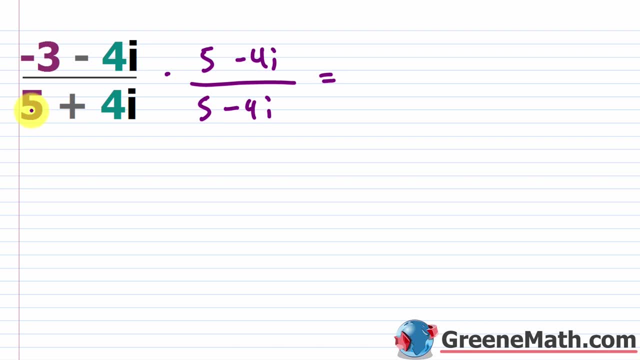 So in the denominator- here again I can just take this guy- Five would be squared, That's 25.. Then, plus this, four would be squared, That's 16.. So this ends up being 41.. Okay, So that's the denominator now. 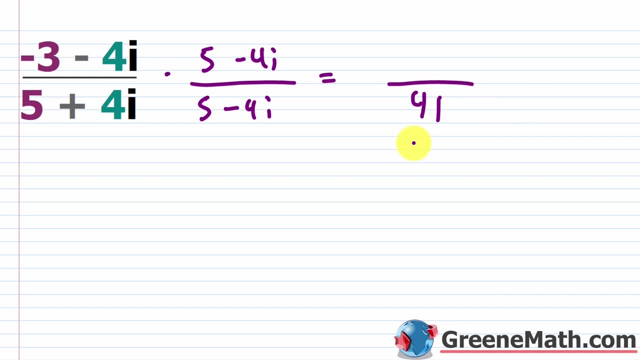 So we're good there. In the numerator you go through and just do four, right. So negative three times five is negative 15.. The outside would be negative three times negative four I, which would be plus. we'll go ahead and say 12 I. 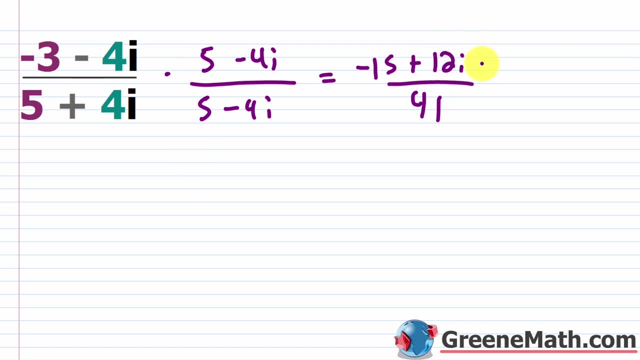 The inside would be negative four I times five, which would be negative 20 I. Let's just go ahead and combine like terms. This would be a negative eight I, so a negative eight I. So I'll put minus eight I there. 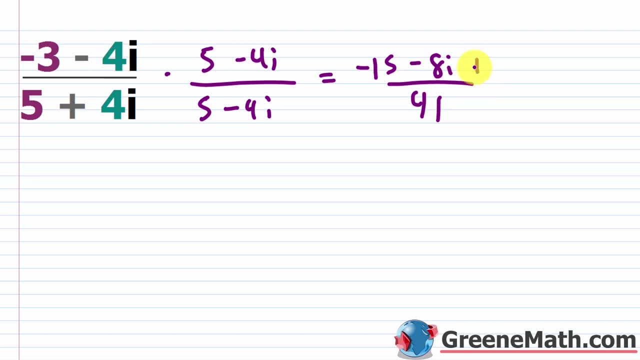 And then, for the last, you have negative four. I times negative four I. That's going to be plus 16, I squared. I squared is negative one. So let's get rid of this and just change the sign. So basically, I have negative 15 minus 16.. 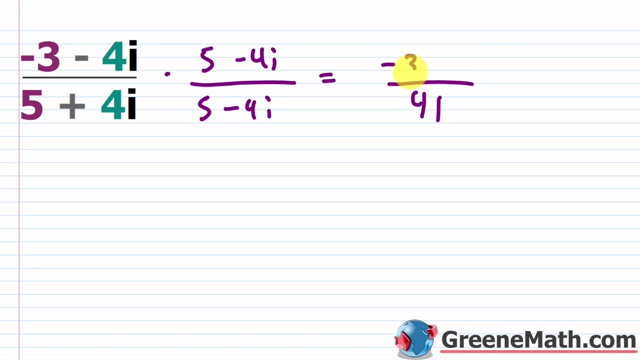 So let's say this is negative 31.. So the top here is negative 31, and then I'll put minus eight. I Okay Now, of course, if you want to write- this is standard form- you want to break this up and say that you have negative 31 over 41.. 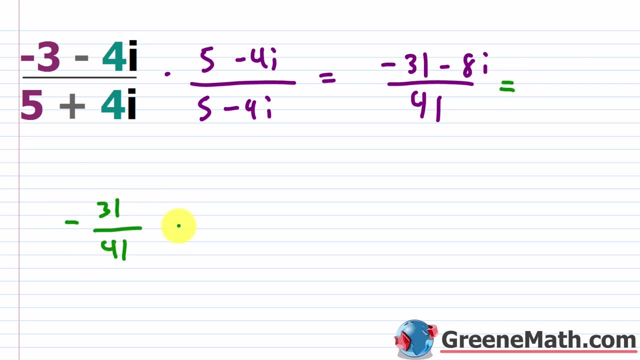 Let me put equals here, So this is the real part, And then we'll put. you put plus negative, or you just put minus. I'll put eight over 41, like this. Okay, Let me make that one a little bit better. 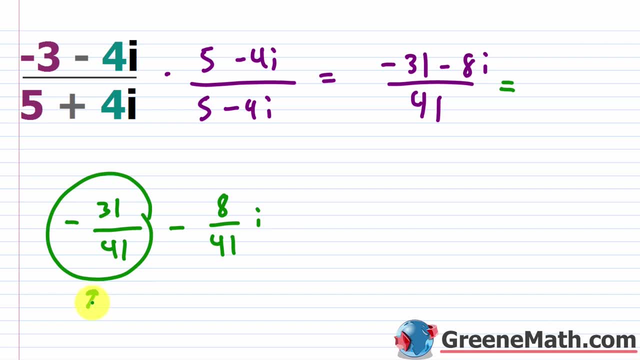 And then I'll put my I out here. Okay, So this is your A or your real part, And then this is your B. Okay, Or your imaginary part. Okay, Then you have your imaginary unit I, And of course you could put plus negative there if you want to. 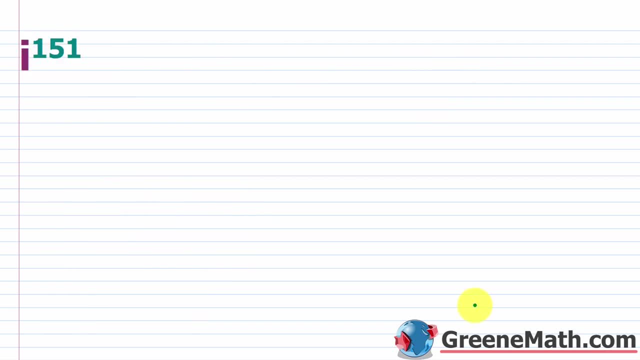 That's up to you. If you put minus there, it's really the same thing, So that's why I'm putting that. Okay, Let's talk about simplifying powers of I, which is a really easy concept Once you realize you go through this little cycle. 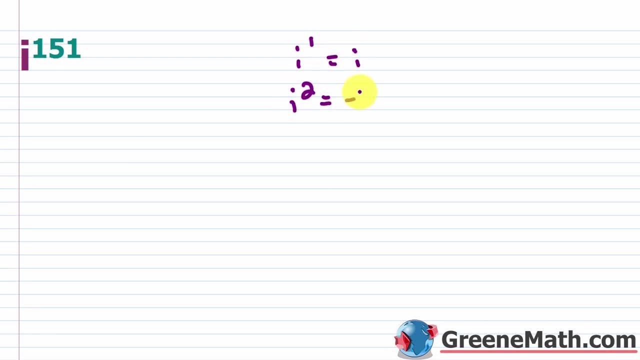 So I, the first power, is just I. I squared is equal to negative one. I cubed is I squared times I right, So this is negative one times I, which is negative I. And then I to the fourth power: is I squared? 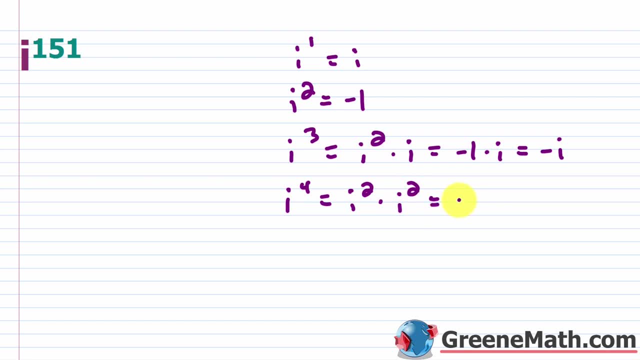 Let me make that better. So I squared times. I squared, which is basically what: negative one times negative one, which is one. Now, using this pattern, it's really easy to rewrite things. Okay, In terms of one of these guys right here. 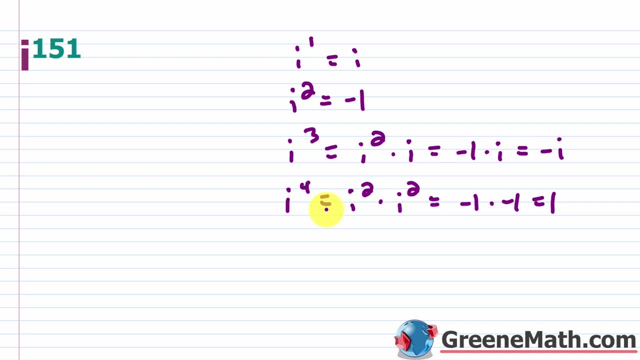 And then you're just going to simplify. Okay, You can put that as your answer. So this involves the rules of exponents. So what I'm going to do here is I'm going to look at this right here. So this number is 151.. 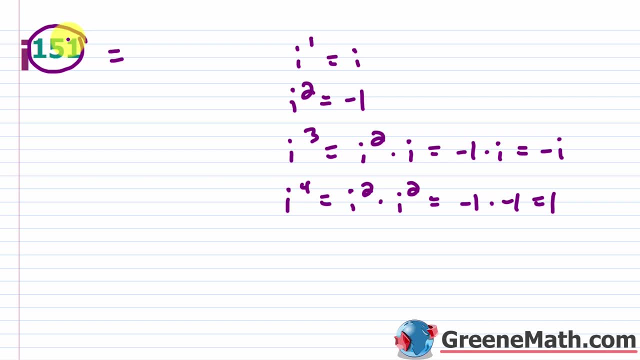 Okay. So thinking about what number going down would be divisible by four. So I just take 151, punch this into my calculator. divided by four gives me one. Where are you going to get 36?? Okay, So 37.75, but I'm going to write this as 37, with a remainder of three. 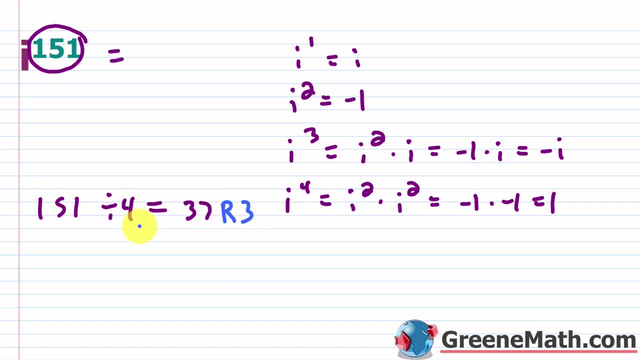 Okay. So basically, the three divided by four is where you're getting the 0.75.. 37 times four is 148.. So I can use that to my advantage. I can say: well, this is I to the power of 148 times I to the power of three. 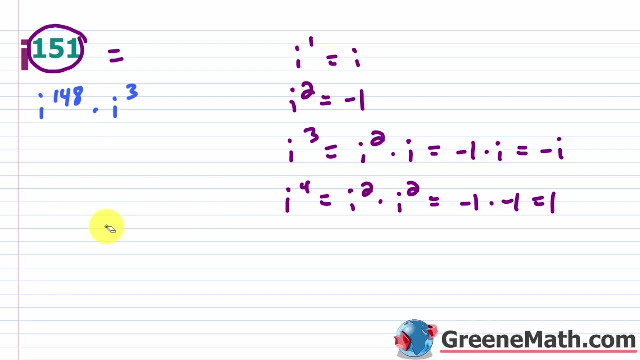 So this is completely legal, right. I basically have just used my rules of exponents. We have I and we have I. So the same base. we would add exponents. We'd be right back to where we started. Now, What I can do, since this number right here is divisible by four, I can use a little trick. 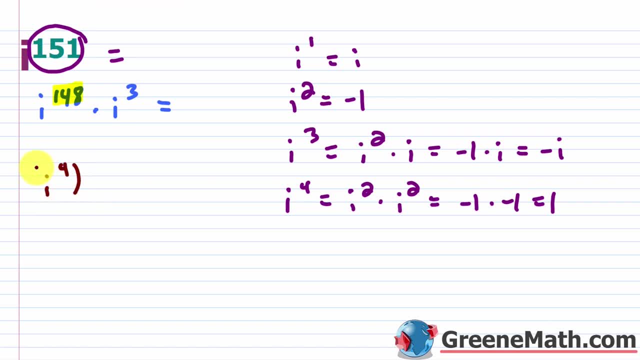 and I can say power to power, rule. I to the fourth power, raised to the 37th power, because again, 148 divided by 37 is four. So four times 37 will be back to 148, right, This is power to power rule. 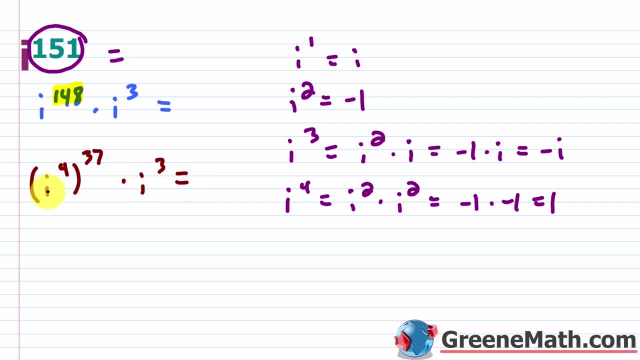 Then times I cubed: Okay Now, why does this work? I to the fourth power. we see over here is one. So this guy, right here is one, raised to the 37th power. one to the 37th power. One to any power is always one right. 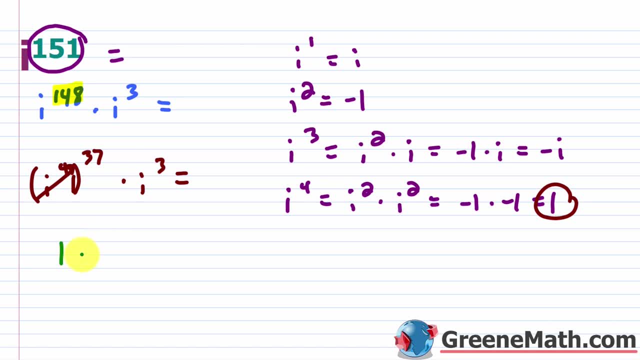 So I can basically just get rid of this and say: this is a big fat one. now times I cubed. Okay, So I've dealt with that, and now I can just go to my little reference here and say, well, what's I cubed? 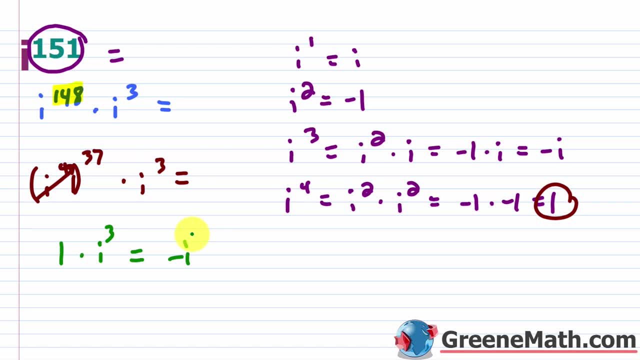 It's negative, I Okay. So that's basically what you want to do when you have a problem like this. when this guy's positive, I still get another example. So we have I to the power of negative 38.. So there's a really easy way to do this, but let me do it the slow way first. 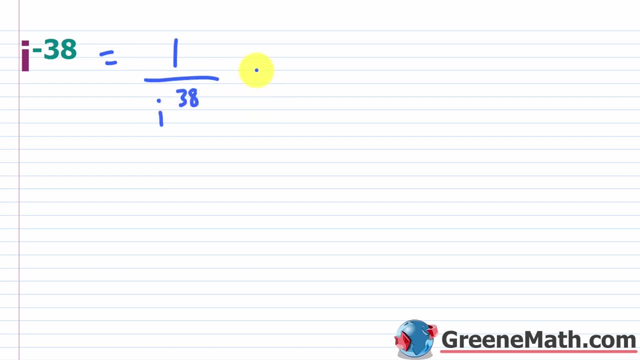 I'm going to write this as one over I to the power of 38.. Okay, Okay, And then of course, I can just do 38 divided by four and see where that puts me. It's going to be nine, with a remainder of two or 9.5.. 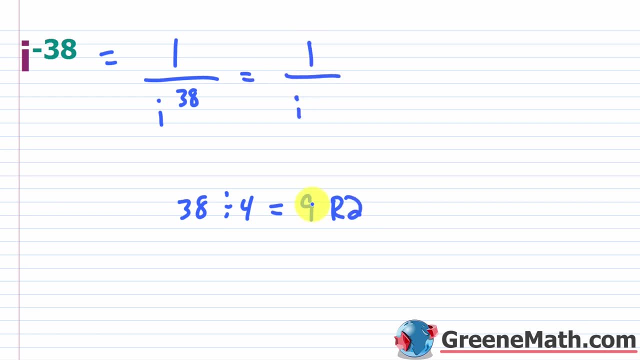 So really I could write this. I could say this is equal to one over I. I'm going to go ahead and put I to the fourth power raised to the ninth power. Okay, Then I'll put times one over. We'll go ahead and say I raised to the power of two. 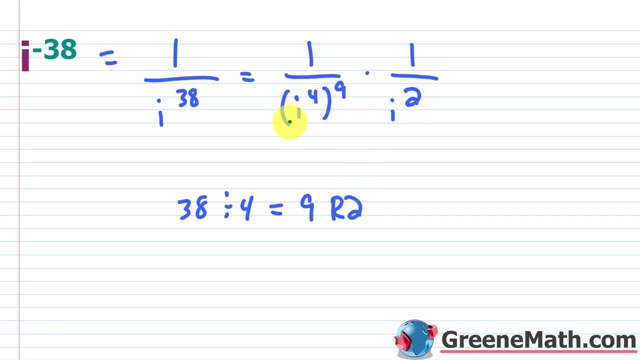 Okay, That remainder right there. Now we know that this guy right here is one and one to the ninth power is one, So I can just keep going like this and say: this is what this is one times one over I squared. I squared is negative one. 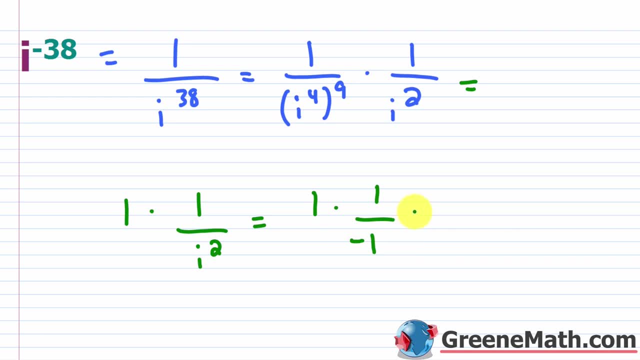 So I can say this is one times one over negative one. So this just ends up being negative one Okay. So really easy to simplify this, but this is kind of a long way to do it. The shorter way if you're working with a negative exponent like this: 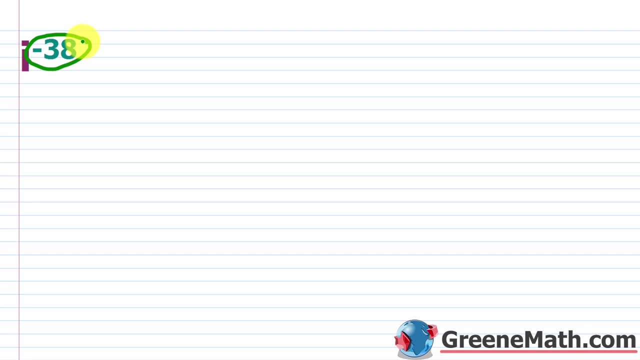 Well, now, what I'm doing is I'm thinking about the smallest number that's divisible by four. Okay, That's going to be larger than this number, And I'm thinking about this in terms of its absolute value. So, if you think about just the number 38, okay, going up, okay. 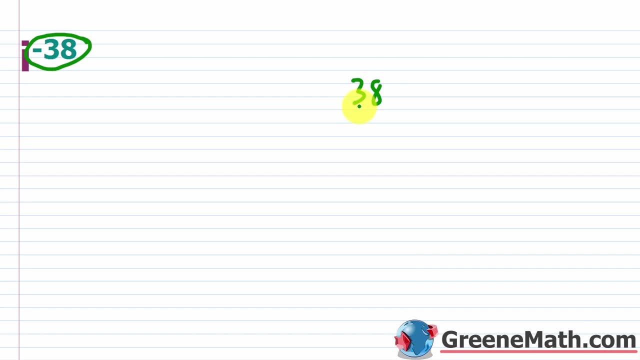 What's the closest number that's going to be divisible by four? Well, it's not 39.. It's going to have to be 40.. Okay, So, in other words, I would want to multiply this by. I would want to say: 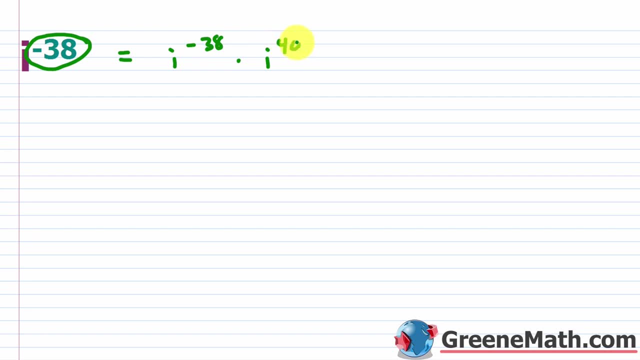 I to the power of negative 38 times I to the power of 40.. That's all I need to do, because what's going to happen here is that I to the power of 40 is just one. I can multiply anything by one. 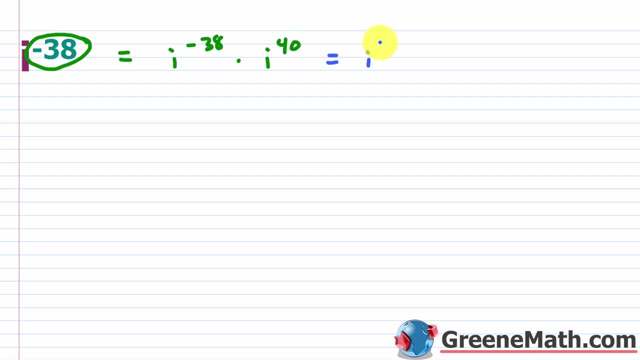 It's unchanged. So this is going to end up telling me that I have what I to the power of negative 38.. Negative 38 plus 40.. Okay, Which is I to the power of two, or I squared, which, by definition, is negative one. 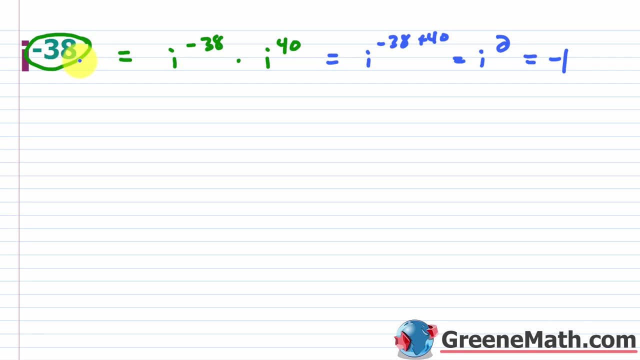 So for me this is a little bit quicker if I get this type of problem, But you can do it the other way if you'd like, All right. So the last thing I want to do is review a few things about the complex plane. 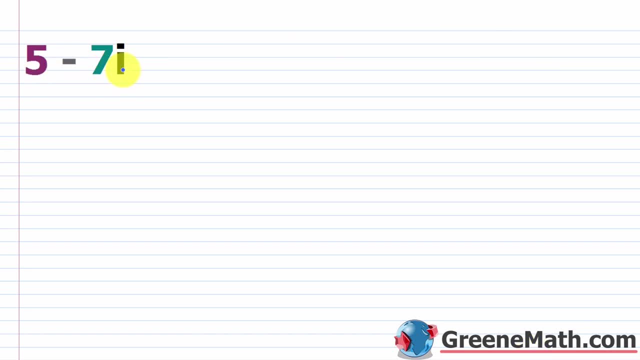 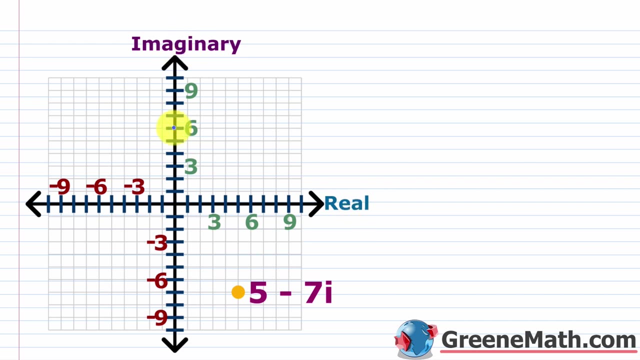 So let's say we wanted to graph something like five minus seven I. What we do is set up a little complex plane. So instead of having X and Y, we now have the imaginary, which is vertical, and the real, which is horizontal. 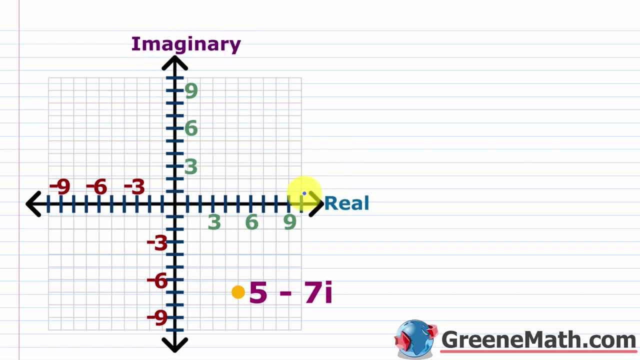 Okay, So before this is X and this is Y. Now, this is imaginary, This is real. Okay, So if I have something like five minus seven, I Well, again, this is the real part. Talked about this earlier And then this right here, the seven is the imaginary. 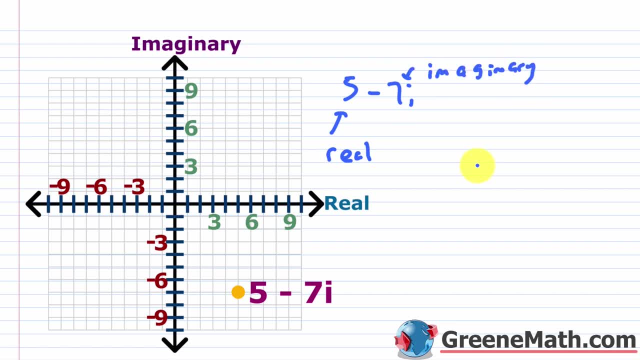 The imaginary part. So all I need to do is move five units horizontally. Five is positive, So moving to the right. So I'm going to go one, two, three, four, five. So right there, And then I want to move seven units down vertically. 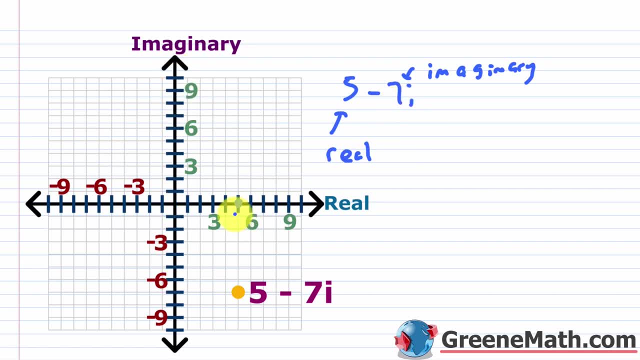 Okay, So I want to move seven units On the imaginary axis going down, because it's negative seven. So one, two, three, four, five, six, seven, And it's going to put me right there. Okay, So this is going to be my five minus seven. I plotted on the complex plane. 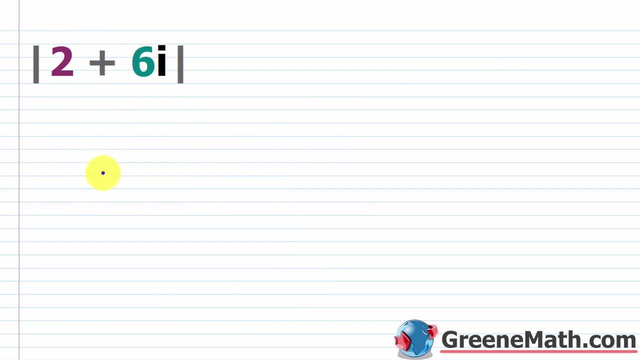 Okay, So the last thing would be the absolute value of a complex number. So if we have something like the absolute value of two plus six- I Again remember the way you would do this- This is going to be the distance between this number and zero, or the origin on the complex plane. 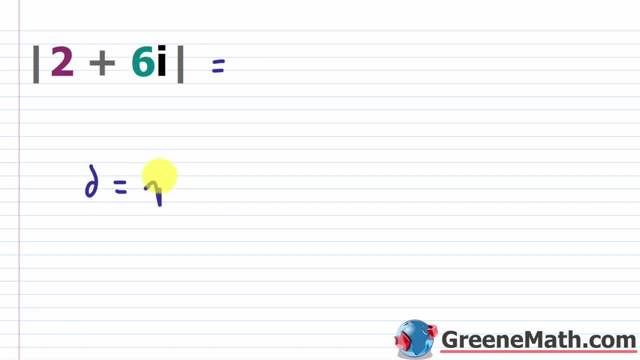 Okay, So your distance formula Normally Is what it's the square root of. You have X sub two minus X sub one quantity squared. Plus you have Y sub two minus Y sub one quantity squared. Well, one of the points is at the origin, right? 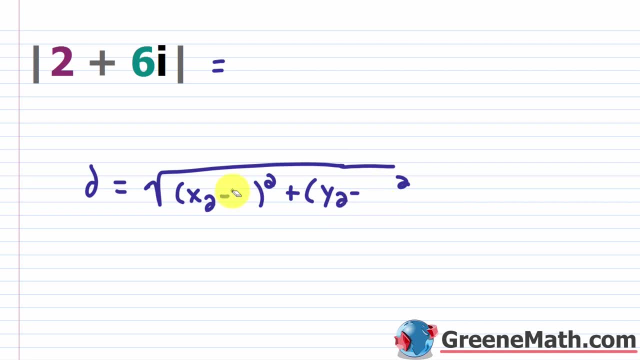 So it's zero, comma zero. So this is zero and this is zero. So this is zero and this is zero. So really I can simplify this and say: the distance between this guy, The origin is the square root of drop the X of two and just say X squared. 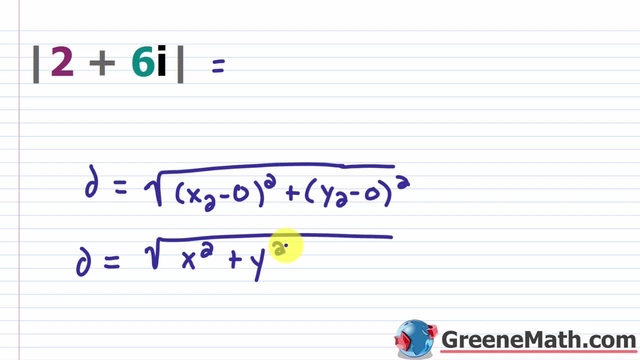 Plus, drop the Y sub two and say Y squared. Okay, Now, in the terminology of Complex numbers, instead of saying X squared, I'm going to say a squared. Instead of saying Y squared, I'm going to say B squared. 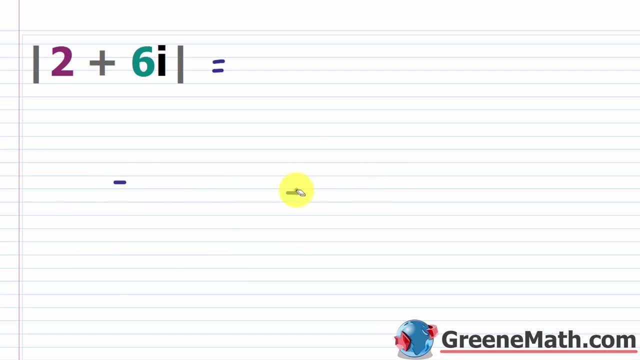 Okay. So what I'm going to do is say That the absolute value of some complex number, let's say a plus bi, is equal to the square root of a squared plus B squared. So this is the square root of two squared. Okay, Two squared. 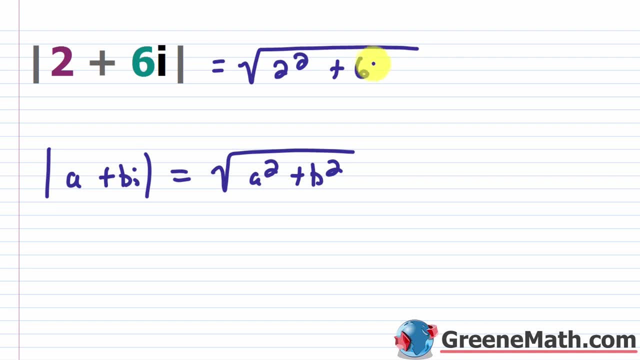 And make that better: Two squared Plus this guy would be six squared, So this is the square root of four plus thirty six, So it's the square root of forty, Okay, Which is square root of four times square root of ten, which in the end- let me get rid of this- 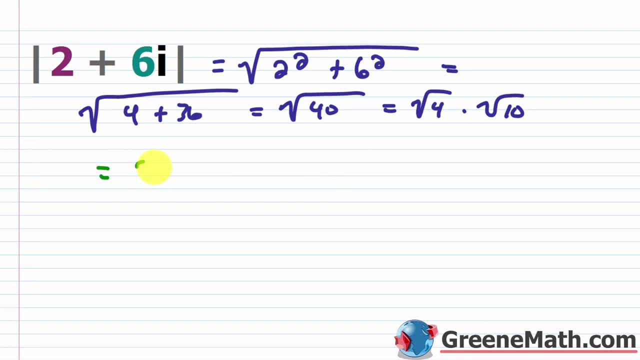 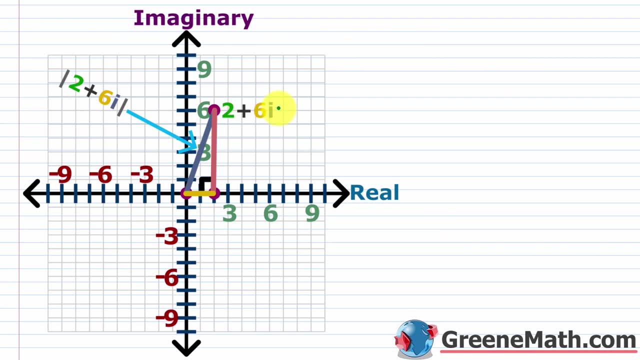 So I have some room to write this And the end is going to be two times square to ten. So this equals two times square root of ten. Okay, If you want to see this graphically, you could plot this guy this, two plus six. I on the complex plane. 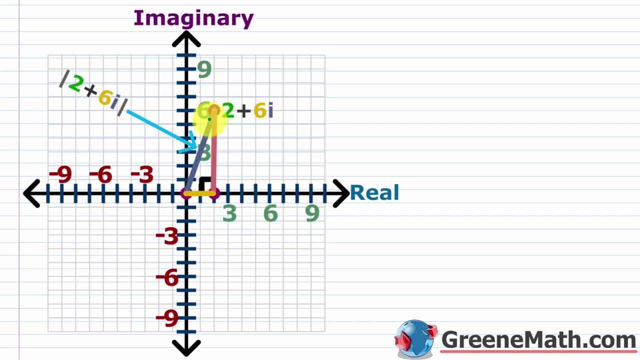 So two units to the right on the real axis, six units up on the imaginary axis. So that gives us this two plus six. I So that's this guy right here, And then basically what I'm doing is just forming a right triangle, right. 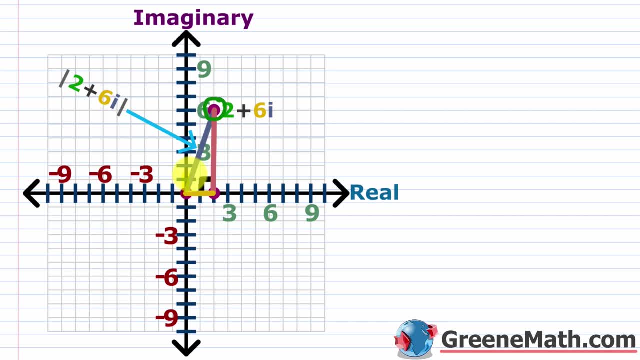 So this guy right here- okay is going to be my hypotenuse, That's what I'm looking for is the length of that guy. So this is the absolute value of the two plus six. I, the absolute value of that complex number. 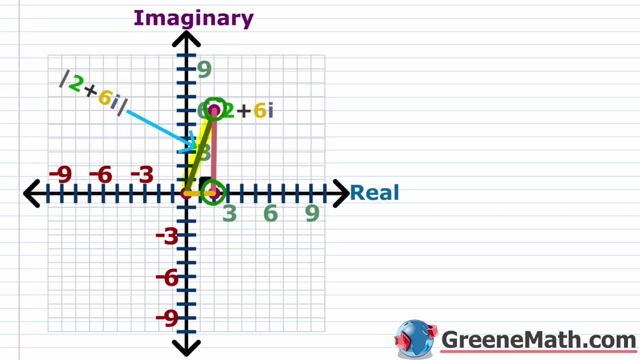 And again, if you look at this distance from here to here, let me circle this in a different color, So let me use this color here. So from here to here, well, this is six units, right? So this is six units. Let me put a six there. 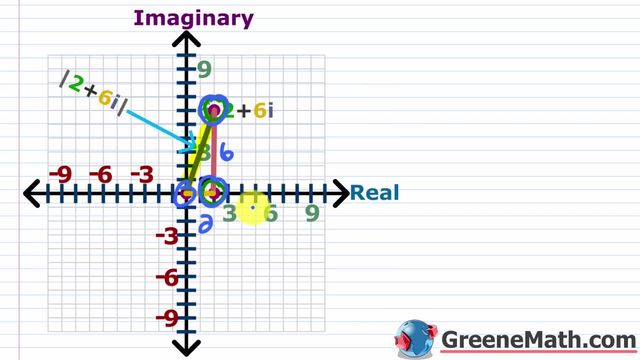 And then if you look at the distance from there to there, it's two units. So again, with the Pythagorean theorem, it's two squared plus six squared is going to be equal to which, in this case, would be the absolute value. 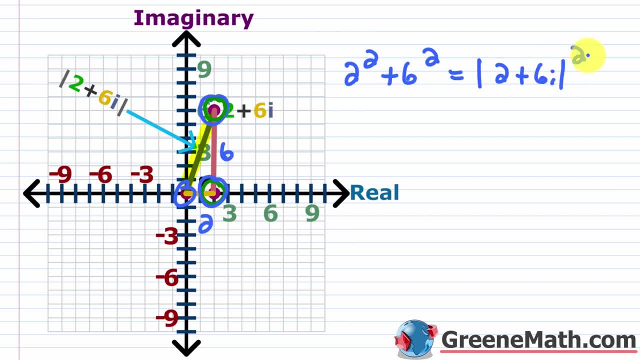 of two plus six. I okay, We might as well just say that's square right. The a squared plus b squared equals c squared. Well, if I take the square root of each side, well then I'm back to my formula. 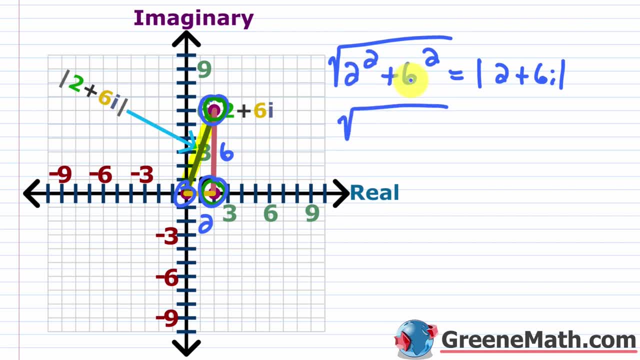 okay, which gives me the square root of four plus thirty six, which is a square of forty. okay, And again, we just simplify that, So we know that at the end, the absolute value of this, two plus six, I is going to be two times the square root of ten. okay, So you can see that graphically. 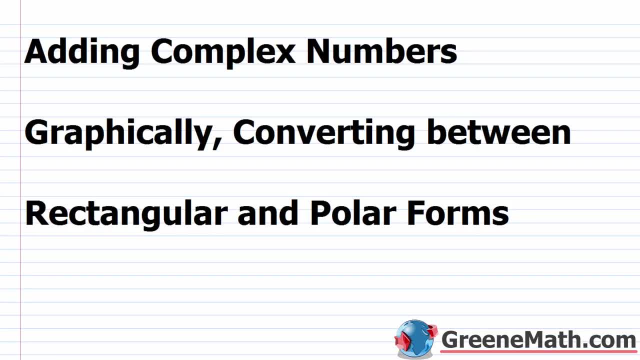 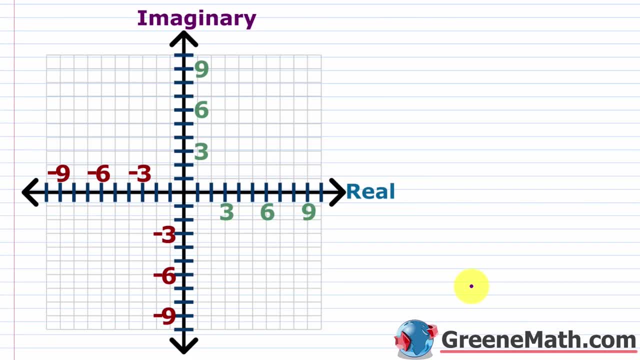 or just from using your formula. In this lesson, we want to learn about adding complex numbers graphically. Also, we'll learn about converting between rectangular and polar forms. Okay, so our first topic of adding complex numbers graphically is very, very easy to do. 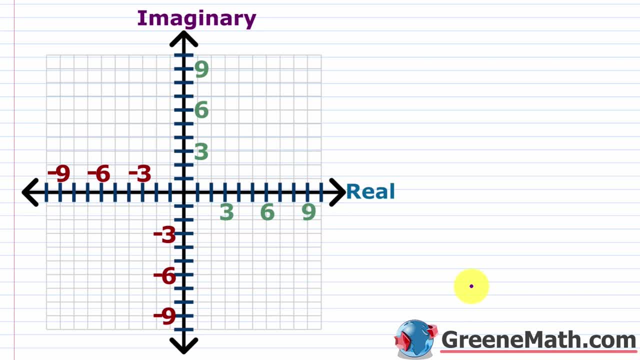 As long as you understand how to add vectors, you're basically good to go. So we return to our complex plane which, remember, is also called the Argan diagram, and basically we replace the x notation here for the horizontal axis with real, We replace the y notation for the vertical axis with imaginary. 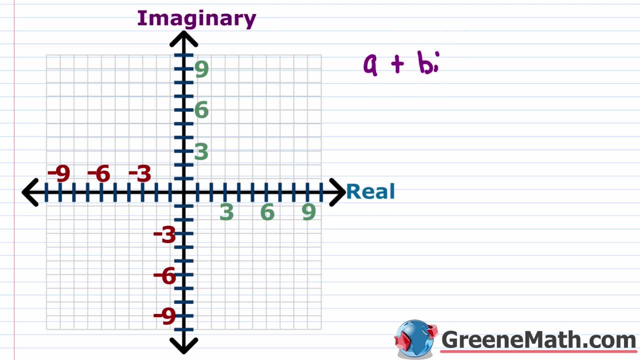 So if you have a complex number like a plus bi- okay, where again the a is known as the real part, okay, and the b is known as the imaginary- the imaginary, okay. part. well, basically, I could use this to plot. 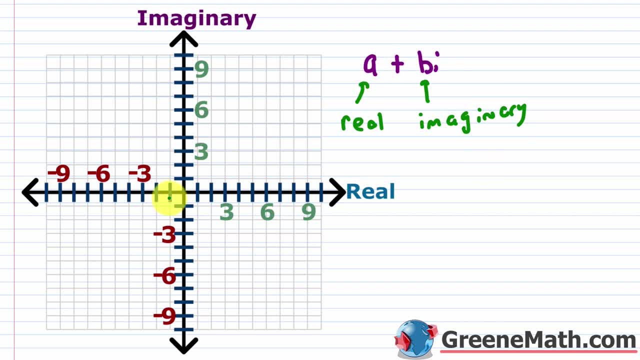 a little point on this complex plane. okay, I'm going to go a units horizontally, okay, and I'm going to go b units vertically, okay. So if I had something like, let's say, three plus seven, i well the coordinates, if you're thinking. 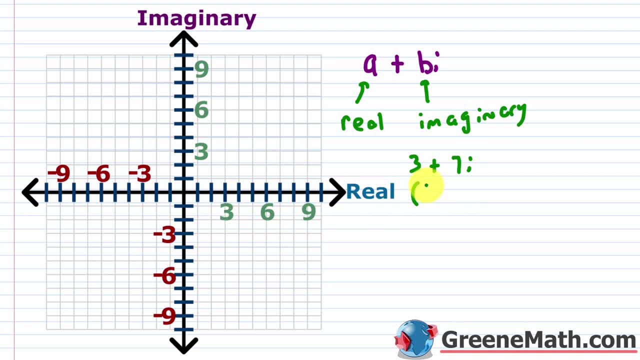 about this as working on your regular xy coordinate plane, where you have some value here, comma, some value here. well, it's three comma seven, right? I'm just moving three units on the horizontal axis- Now it's called the real axis- and I'm moving up seven units, okay. 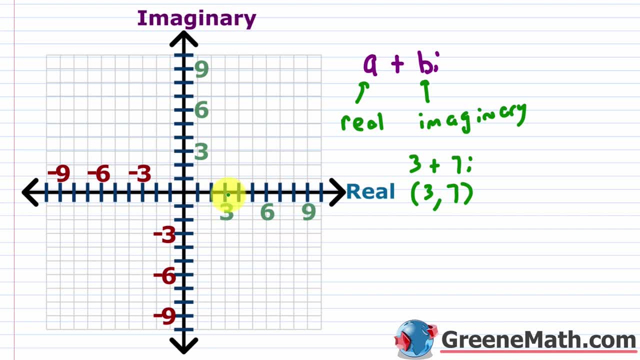 on the vertical axis, now called the imaginary axis. So three units to the right, seven units up would put me right there, okay, So I would go ahead and label this as the complex number three plus seven. i okay If you wanted to do another one. 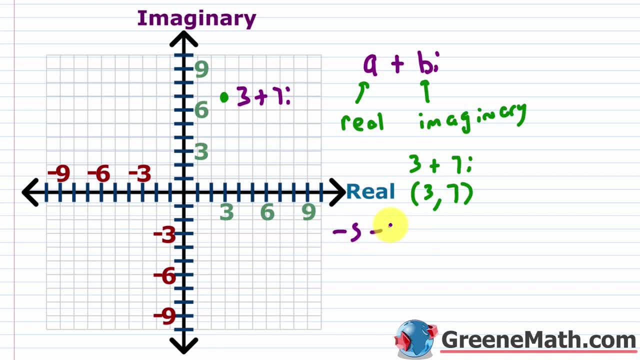 let's say we do something like negative five, let's say minus four, i okay, So the coordinates there would be negative five, comma negative four. So I'm just going five units to the left on the real axis and then four units down on the imaginary axis. 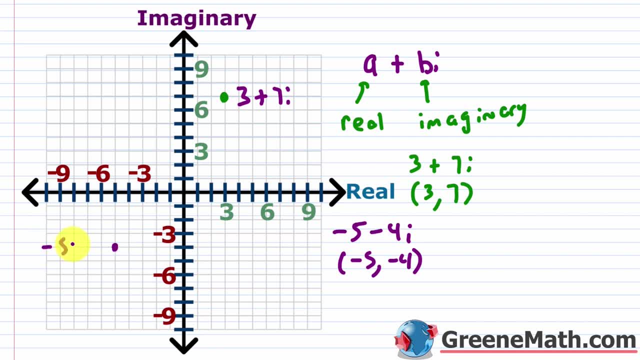 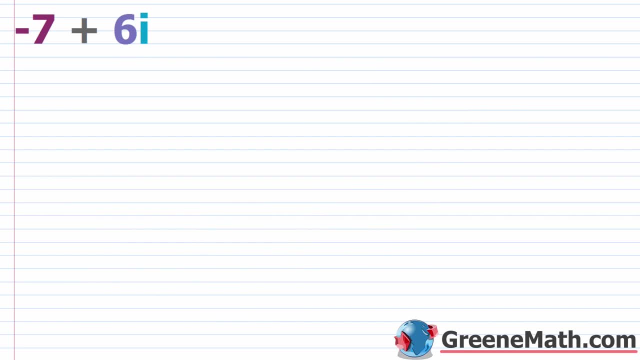 So right about there, let's go ahead and say this is negative five minus four i. For the purposes of making sure that you understand how to do this, you should pull out a sheet of paper and just make a rough sketch of an argand. 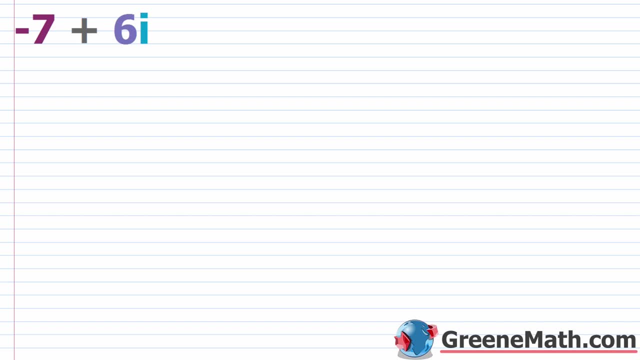 and we're going to use it throughout the lesson, So you might want to have that handy And go ahead and pause the video and try to just graph this guy. Think about where it would be on your complex plane. All right, so hopefully you gave that a shot. 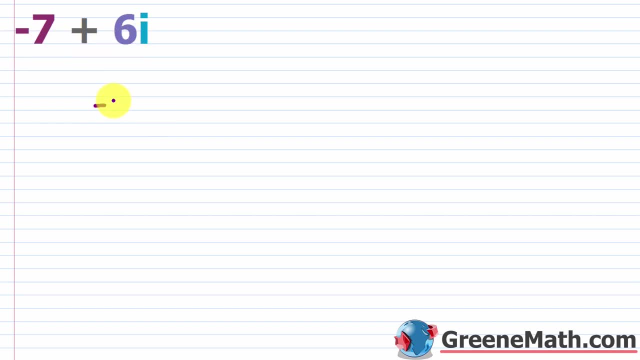 This negative seven plus six, i again the real part's negative seven. So I'm moving seven units to the left. The imaginary part is six, so I'm moving six units up. okay, So seven units to the left, six units up, which would put us exactly right here. 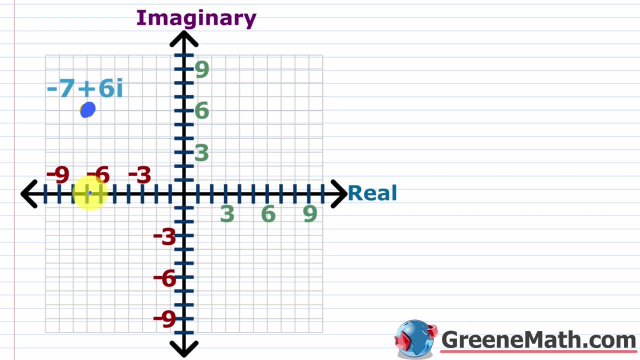 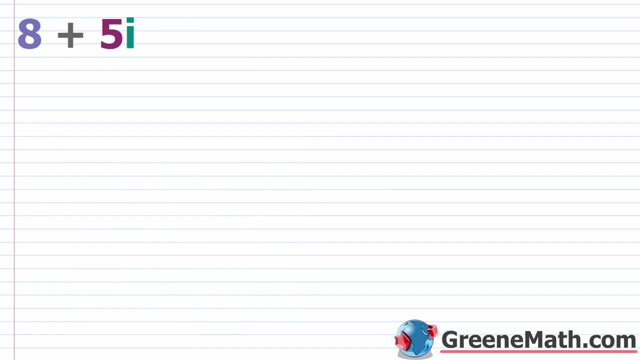 Okay, so this would be your negative seven plus six i, seven units to the left and six units up. All right, Additionally, as you move higher in math, we start to think about graphing a complex number using vectors. okay, And specifically here: 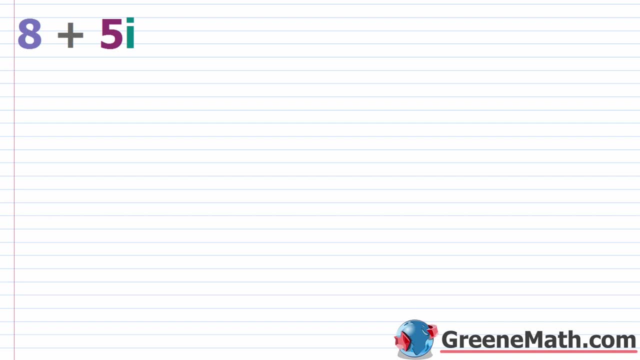 we're going to use a position vector or a vector in standard position. okay, So this just means that the initial point is at the origin. If you think about this in terms of a complex number, your origin is going to be at zero plus zero i. 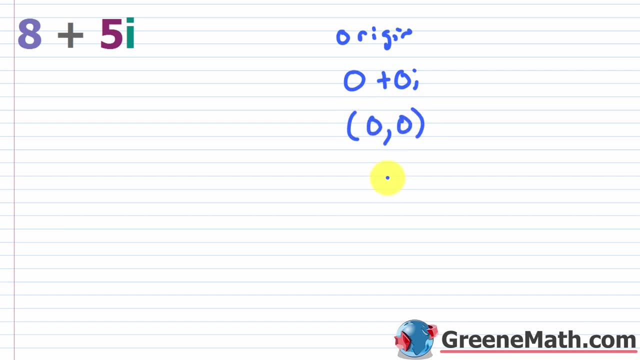 or you could say zero comma zero if you want the coordinates. okay, So the initial point's at the origin and the terminal point would be at this, eight plus five i. So again, it's eight units to the right and five units up. 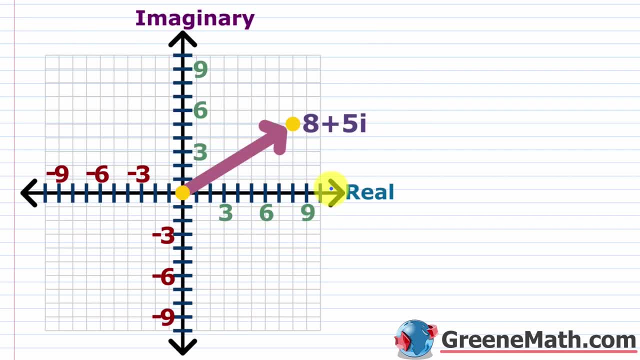 Let's see this position vector graphically. So this would look something like this: Your initial point is at the origin, So right there, your terminal point is at eight plus five i. So again, you're just going eight units to the right and then five units up. 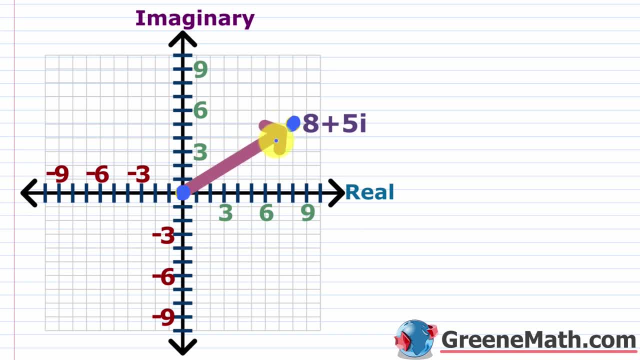 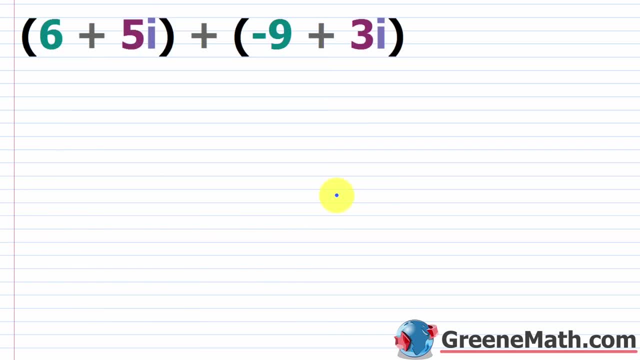 And you have a directed line segment or a vector. Okay, so this is how we're going to show this eight plus five i when we're asked to graph it as a vector. All right, so now let's use the fact that we can graph a complex number. 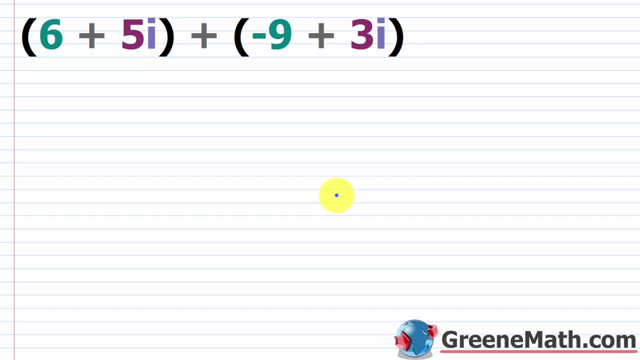 as a position vector to show the sum of two complex numbers graphically. okay, So we have this: six plus five i, plus negative nine plus three i. Let's just add this together real quick, just so we know what we're supposed to get. 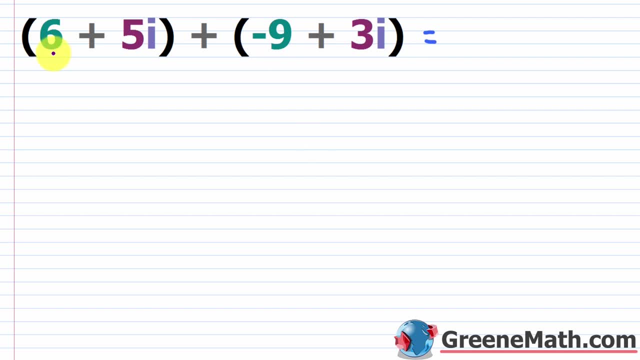 And then we'll go to the coordinate plane. So we know we would add the real parts. So we do six plus negative nine. Okay, that's your first step. Then plus we would add the imaginary parts, So five plus three, okay. 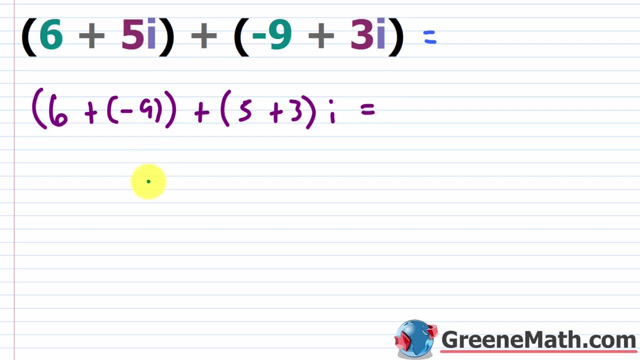 And this is multiplied by the imaginary unit i. So what I want to do here is: do six plus negative nine, That's negative nine, That's negative three, And then, plus, you have five plus three, which is eight, and then times the imaginary unit i. 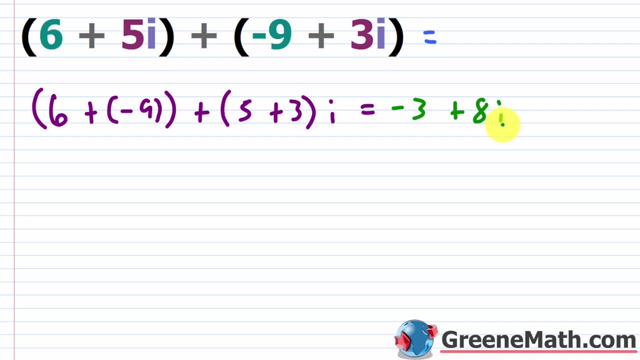 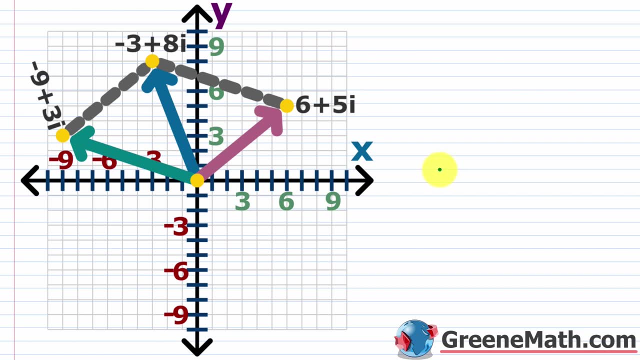 So negative three plus eight, i is your resultant vector. Okay, so let's look at this graphically. And again, you can do this with the parallel aquarium method or the triangle method, whatever you want to do, But essentially you'll see here that we have the origin here, okay, 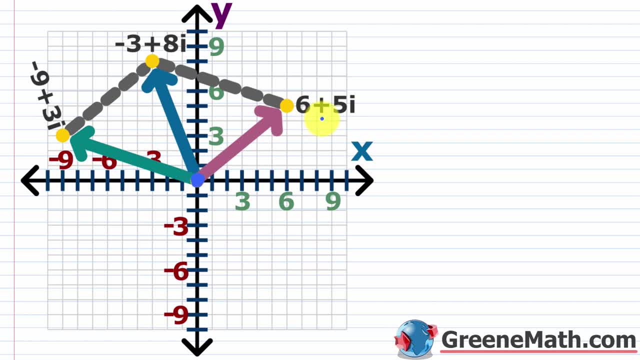 which is our initial point for basically everything. Okay. so the six plus five, i let's say you sketch that first. So here's the terminal point. Then you have this negative nine plus three, i Okay, so if we sketch that guy, that's the terminal point. 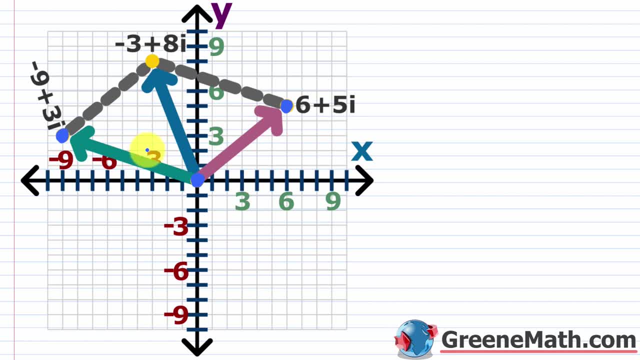 And then again, if you want to do the parallelogram method, this guy gets shifted down to make this side here- okay. to make this side here, This guy gets shifted down to make this side here, okay. And this point right here is going to be your terminal point for the resultant vector. 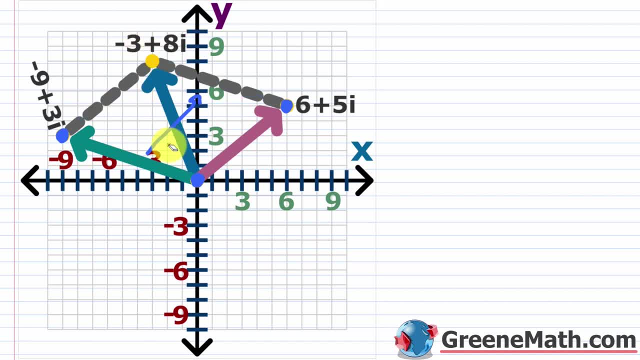 You see, you get the negative three plus eight. i Again, if you want to use the triangle method, you can do that as well. Basically, you're going to shift this guy down here, So you would have that vector. You're going like that, okay. 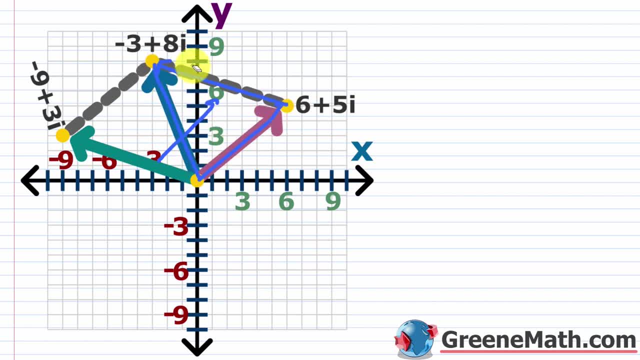 And you would have your triangle looking like that. okay, So, whatever you want to do, you can just show this graphically. I prefer this method because this is what's shown in most textbooks And basically, you're keeping in line with the fact that this is a position vector, and this is a position vector. 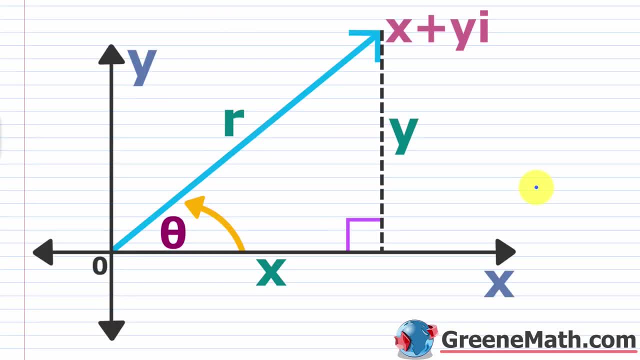 And then this is your resultant vector. All right, So what we want to do now is move into writing a complex number in what's called the trigonometric form, also known as the polar form. okay, So typically we see our complex numbers written as a plus bi. where, again, 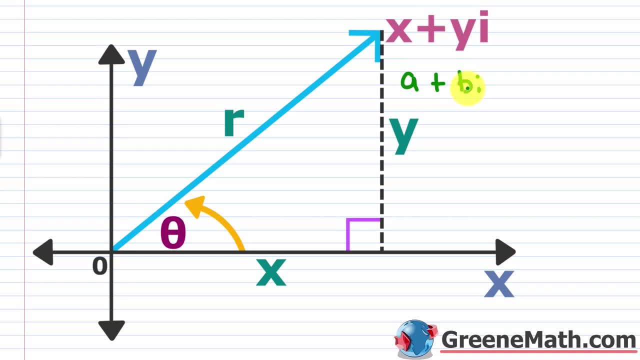 the a is the real part and the b is the imaginary part. or some books will say bi is the imaginary part. So what we're going to do is just switch this over to the x plus yi, where x is now going to be the real part. 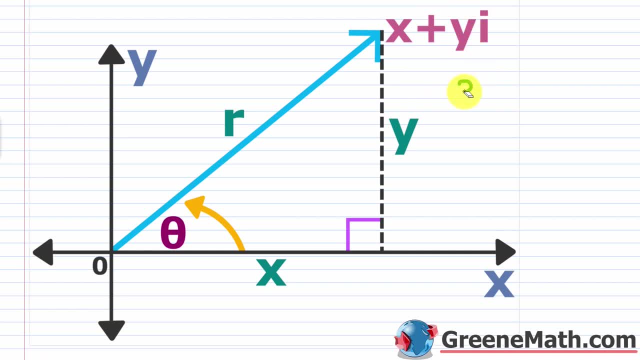 and y is going to be the imaginary part. Now, in terms of notation, you're going to sometimes see that the i is switched, So you might see x plus i times y. This is done for clarity. Sometimes you'll have a radical involved. 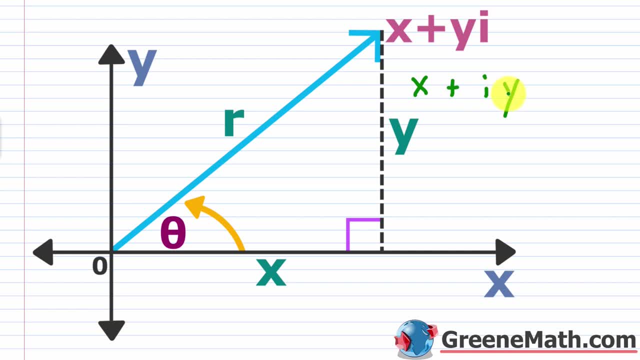 So you just have to be very, very careful when you have i written like this to understand what the imaginary part is. okay That i is always separate from that. You have to remember that And I'll show you that specifically here with some examples. 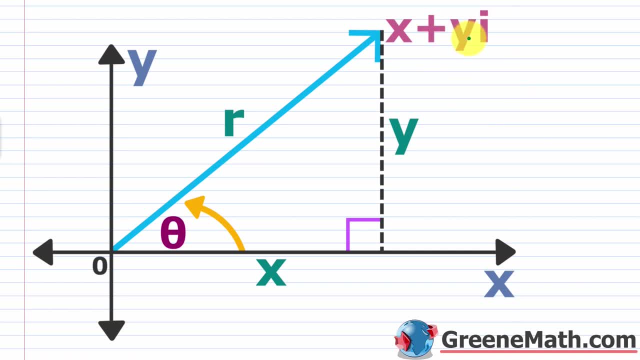 Now, in terms of getting this guy from what we call rectangular form, which is the form that you normally see it in the a plus bi or the x plus yi- into this polar form, you need to consider a few things. So we've graphed this guy. 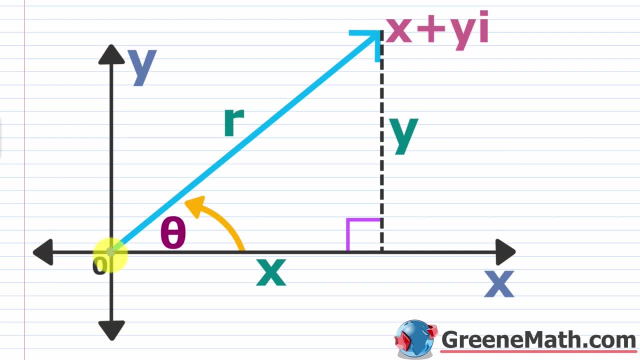 I as a vector, a position vector to be specific. So the initial point is at the origin zero comma zero. The terminal point is at the complex number x plus yi, where you could say the coordinates here are x comma y on the complex plane. 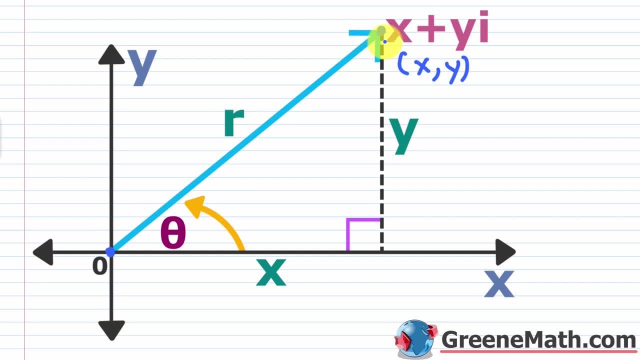 So if you think about a few things, first off, the length or the magnitude of this vector is labeled as r. We've seen this a bunch of times where we think about: OK, well, the length of this guy is the absolute value of the complex number. 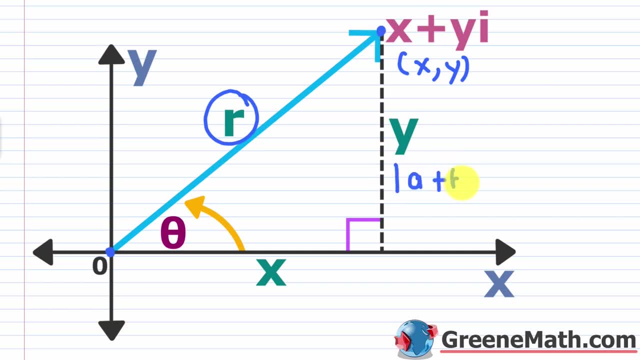 OK, Going back, Like we said, the absolute value of a plus bi is the square root of a squared plus b squared Again. this is just the Pythagorean theorem, right? If I go through here and I think about how to get the length of this r or the magnitude of this vector. 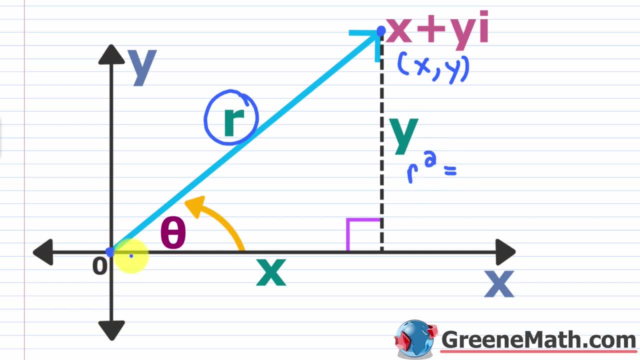 well this guy here would be: r squared is equal to the length of this, which is x, So x squared plus the length of this, which is y, So y squared. a squared plus b squared equals c squared. We're just going back to the Pythagorean theorem. 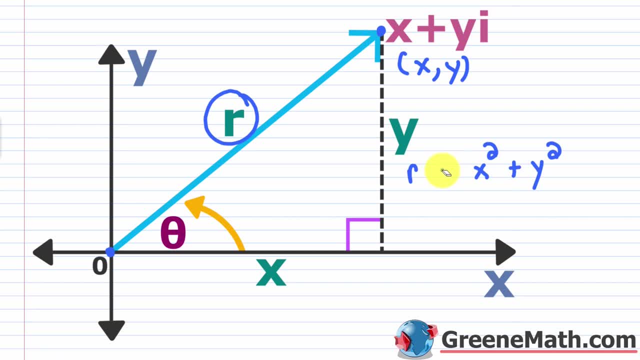 If I take the square root of each side, I get that r is equal to the square root of x squared plus y squared. OK, so this is something we're going to need today. When we want to find our r value. we just use this little simple formula. 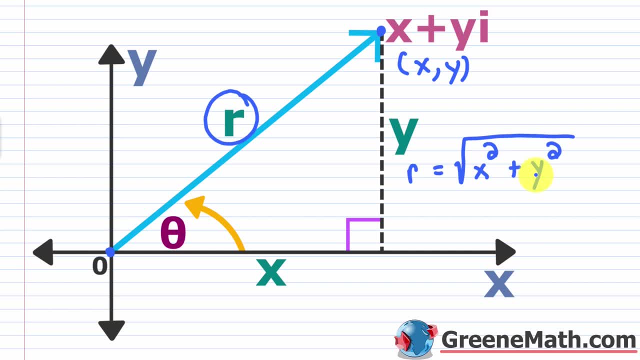 Again, if you can't remember, it's just the absolute value of the complex number. That's all it is. So let's go ahead and cut this away and let's just paste this on this little sheet here. We'll just go back and forth. 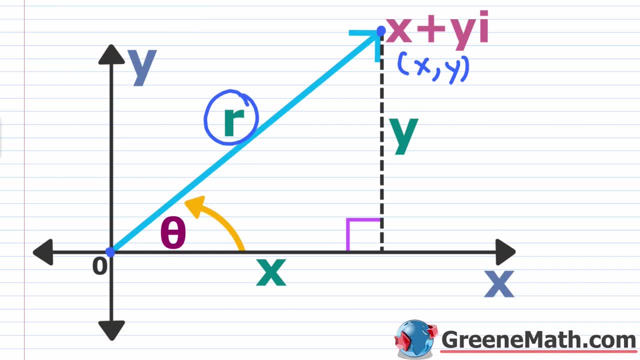 So we also need to know about a few other relationships. So we think about this angle, theta here, this direction, angle for our position here, The cosine of theta is what? So the cosine of theta is what? Remember it's adjacent, which is x, over hypotenuse, which is r. 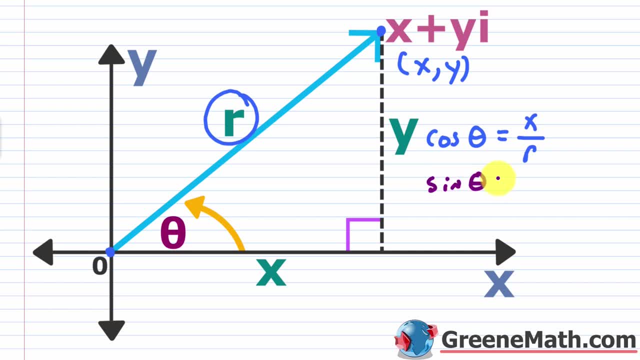 And then we can also say that the sine of theta is what It's opposite, which is y, over hypotenuse, which is r. OK, let's grab these and cut these away and paste these in here Again. we're going to be using this in a second. 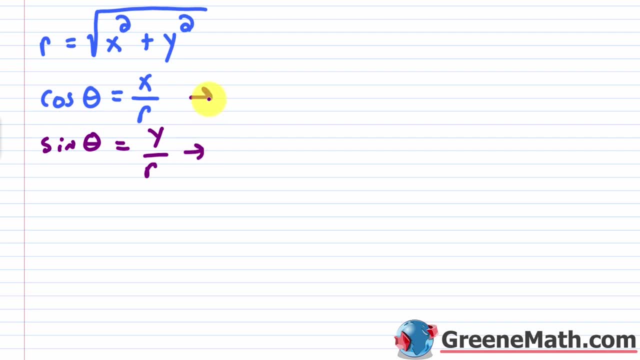 And basically what I want to do is I want to solve these for x and y. OK, So to solve this for x, I would multiply both sides by r and I would have: x is equal to r times the cosine of theta. To solve this for y, I do the same thing. 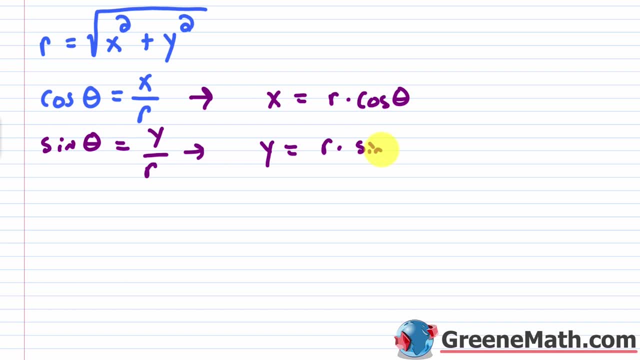 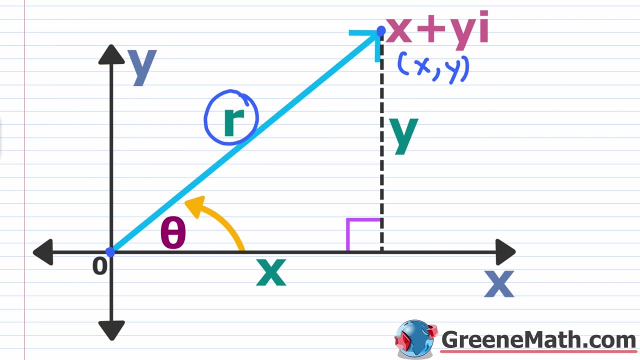 I'm going to multiply both sides by r, So I would have r times the sine of theta. OK, So we're going to use this in a little while. Let's go back up. There's one other thing we need So we recall when we work with vectors. 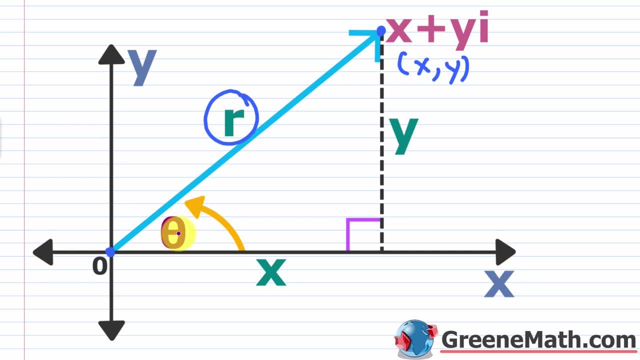 we figure out the direction angle theta using the tangent right. So we say that the tangent of theta is equal to y over x where x is not zero. OK, So we're going to use this as well. But again, you remember from working with vectors. 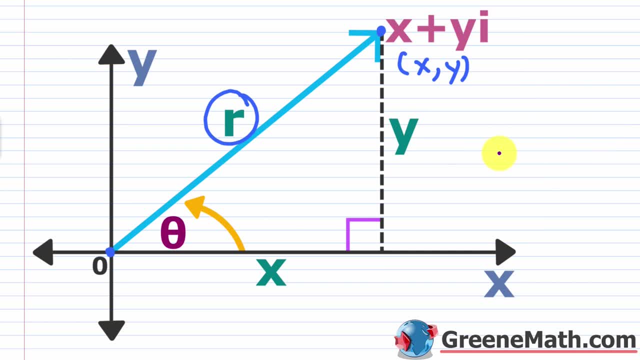 you have to be really, really careful with the inverse tangent function. OK, With the inverse tangent function you're going to get something in quadrant one or four, only One if your argument is positive and four, rotating clockwise, if your argument is negative. 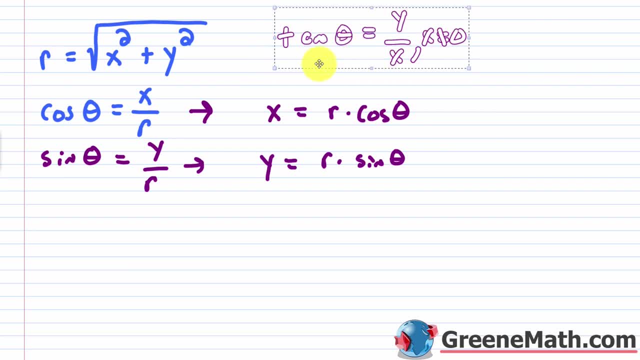 So let's come in here and let's paste this in, And I guess we can put that about right there. OK, So the polar form. let me just start with the rectangular form. So we have x plus yi. If you want to write yourself a little note and say, OK, well, this is a plus bi. 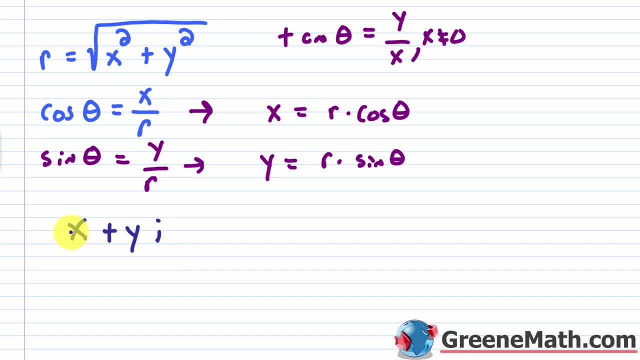 just to keep track of this again: x is the real part, just like a, y is the imaginary part, just like b. it's all. it is Just a little notational change. So this is the standard form or the rectangular. 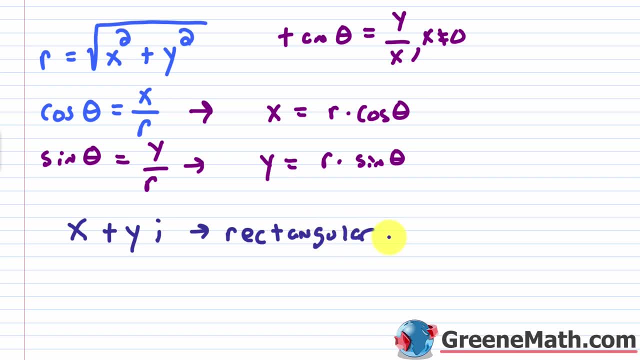 Rectangular. I can never spell that form. OK, Then if you want the polar form, we're going to do a little bit of work, So let me do this on another sheet and I'll actually come back. So we have the x plus yi, and I'm just going to be plugging in for x and y. 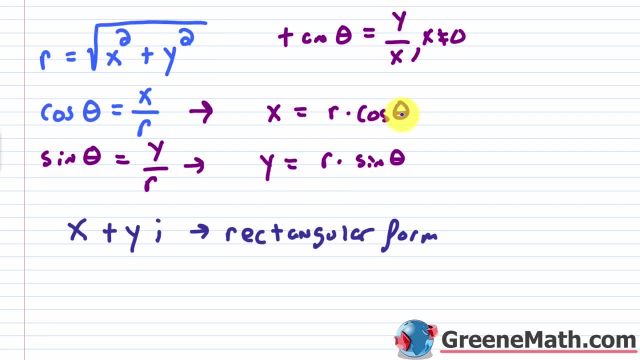 If I go back you see that x is r times cosine of theta and y is r times sine of theta. I'm just going to plug in So r times cosine of theta. r times cosine of theta will be plugged in for x and r times sine of theta will be plugged in for y. 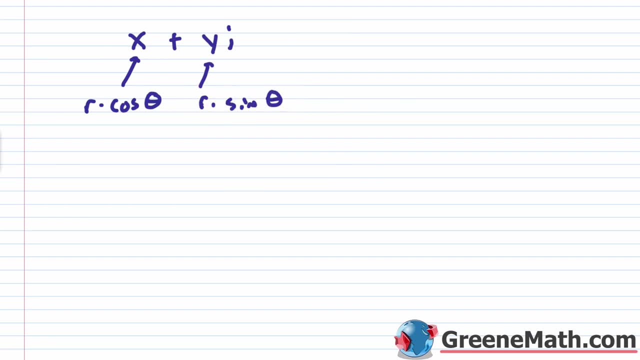 So r times sine of theta. OK, So what I'm going to do here, say this is equal to: I'll have r times the cosine of theta, then I'm going to put plus, I'm going to put r times sine of theta and I'm going to wrap this in parentheses just for clarity. 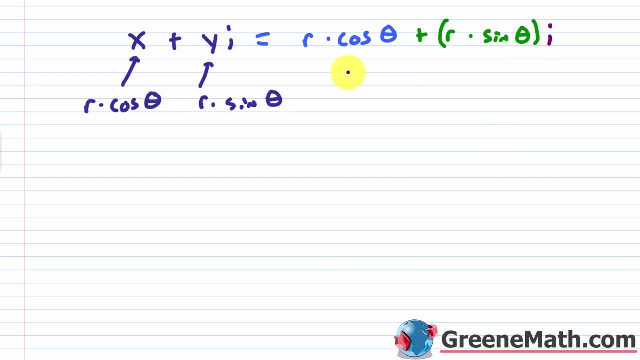 This is going to be multiplied by the imaginary unit. i OK. So again, this is x- this whole thing right here. and then this is y- this guy right here- and it's multiplying the imaginary unit- i OK. So I'm going to go a step further and just factor the r out now. 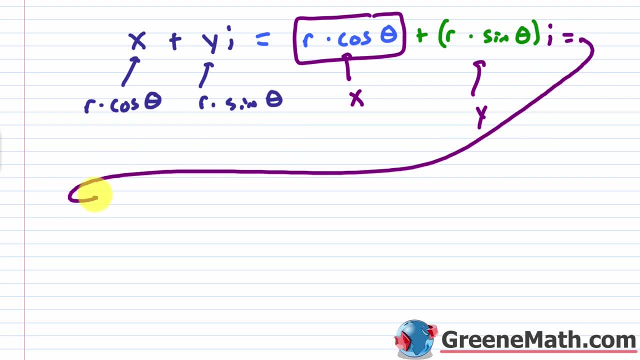 So let me put equals, and I'm going to come down here to this. let me drag a little arrow down here. If I factored out the r, where would I be? I would have r times inside of parentheses. I would have my cosine of this theta. 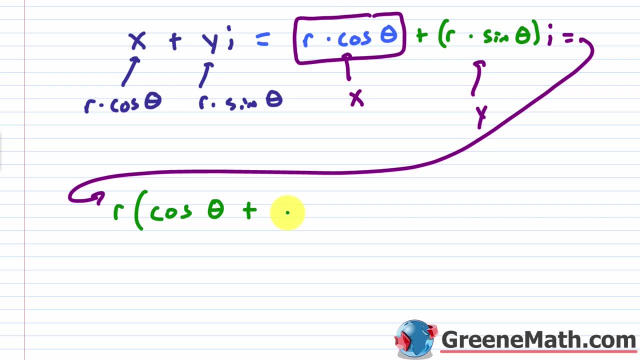 and then, plus again, I pulled out the r. I would have my sine of theta, But what I'm going to do is I'm going to put the i out in front, So i times this sine of theta. OK, And you have to be very, very careful when i is written this way. 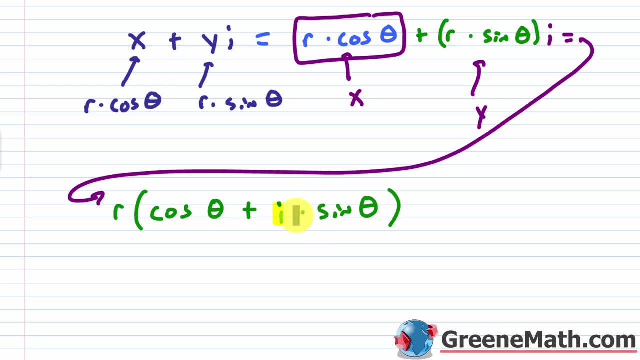 because sometimes it's going to get mixed up, And again I'll show you some examples where you need to be careful of this. OK, So this is your polar form. that's all it is. Some books will abbreviate this and they will put: they will put r times c i s. 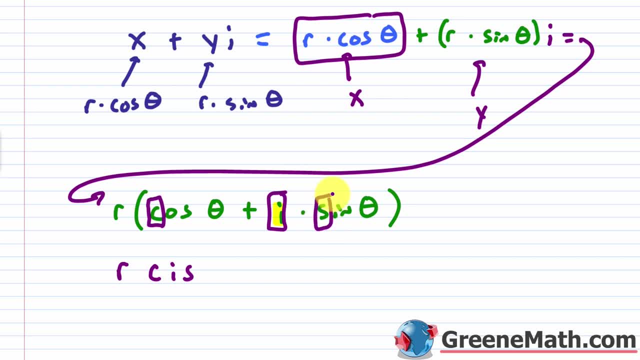 It's an abbreviation, So the c, then you have the i and then the s, OK. So that's how you can remember: r times c, i, s and then times the angle theta, OK. So if you want to write it as r cis theta or write it like this, this is more popular. 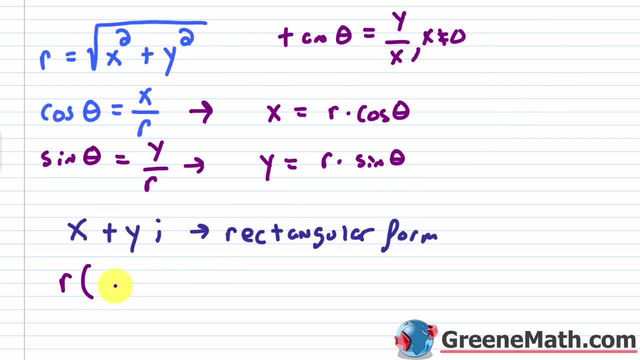 This is your polar form, So let me write this up here. We have r times, you have your cosine of theta plus i times your sine of theta like this: This is your polar form. Or again, some books are going to call this the trigonometric form. 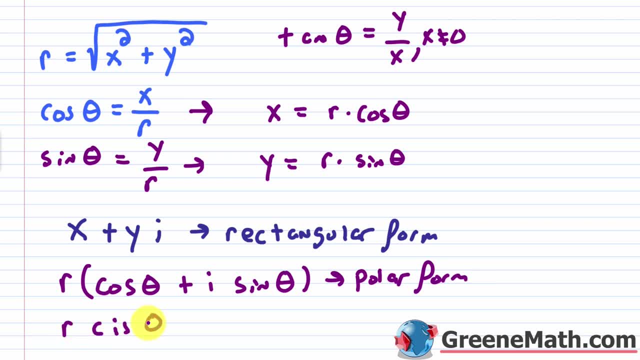 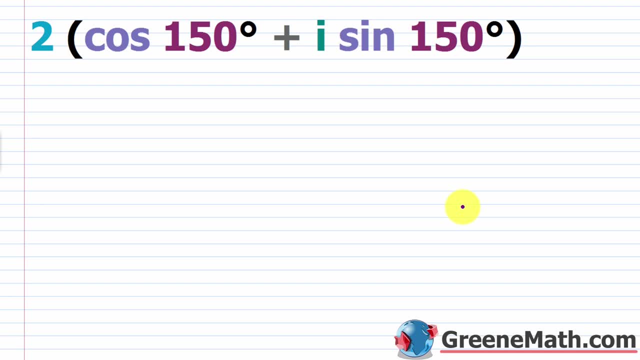 And the shorthand for this is r times cis of theta. All right, let's just look at some examples of converting back and forth between the two. This is a very, very easy process, but you do need to work a few examples so you get used to things, OK. 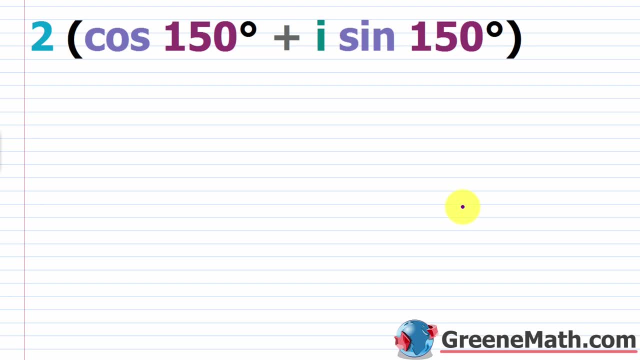 You'll also see a lot of these come up over and over again, because they're using values on the unit circle. So what I have here is 2 multiplied by the cosine of 150 degrees, plus i times the sine of 150 degrees. So this is in the polar form, right? 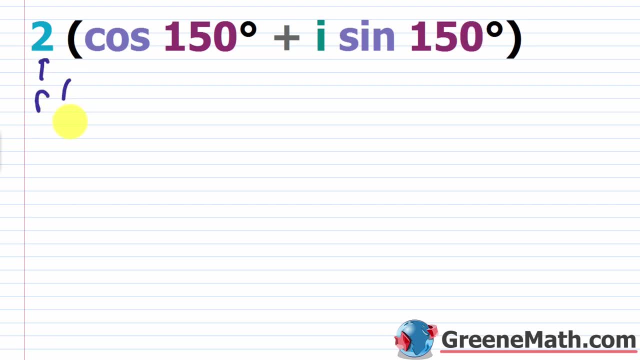 You have some value r here, which in this case is 2, and it's multiplied by cosine of some angle theta. in this case is 150 degrees plus i times your sine of some angle theta. OK, So all I would do here, basically, is figure out what is the cosine of 150 degrees. 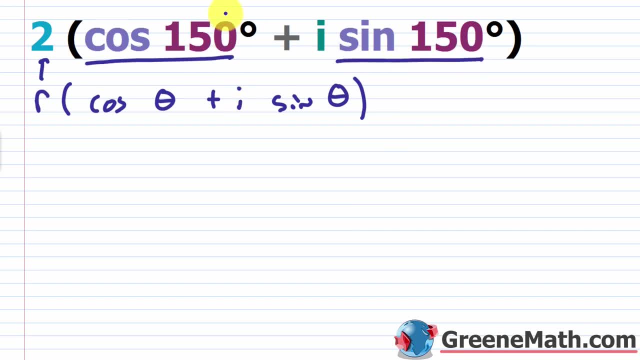 what is the sine of 150 degrees? basically replace things and then use my distributive property to distribute the two into everything and you're going to have the format of x plus yi. OK, just like you want. So, first and foremost, what is the cosine of 150 degrees? 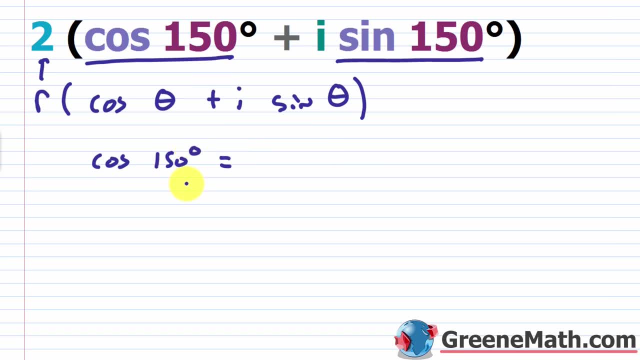 Remember this has a 30 degree reference angle and we're in quadrant 2.. Cosine is negative, OK, And the 30 degree reference angle, cosine of 30 degrees, is square root of 3 over 2.. So I can say this is the negative of the square root of 3 over 2, OK. 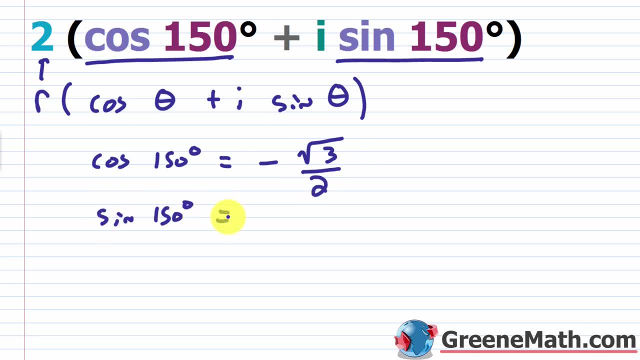 Then the sine of 150 degrees. same 30 degree reference angle, But again I'm in quadrant 2.. So sine is positive. This is going to be one half OK, and positive one half at that. So all I need to do now is just go through and basically replace things. 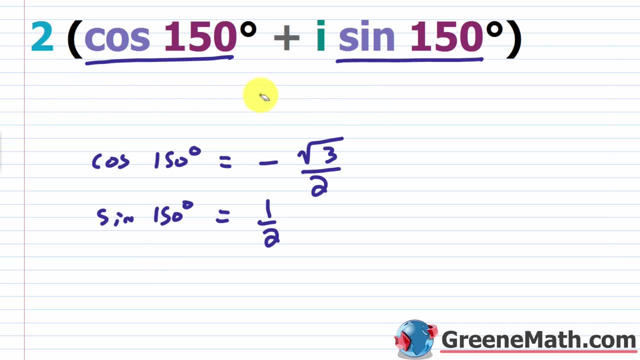 Let me get rid of this. I think we don't need this anymore. I'll say that I have what I'm just going to put equals here. I'll say two times here. I'll put the negative of the square root of 3 over 2 and then plus. 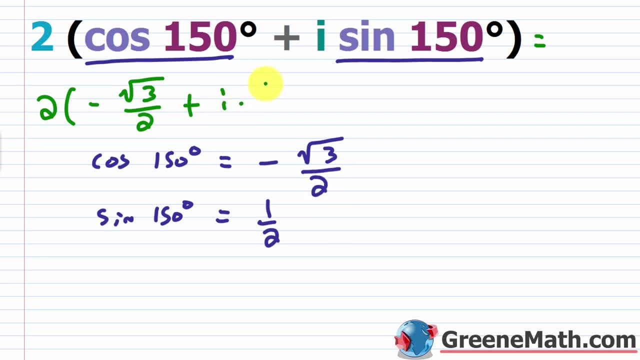 I'm going to put the i here, OK times. I'll put my one half, OK. Be very careful with the i. Again, it gets switched around a lot. Sometimes it's here, sometimes it's there. Just be careful with it. 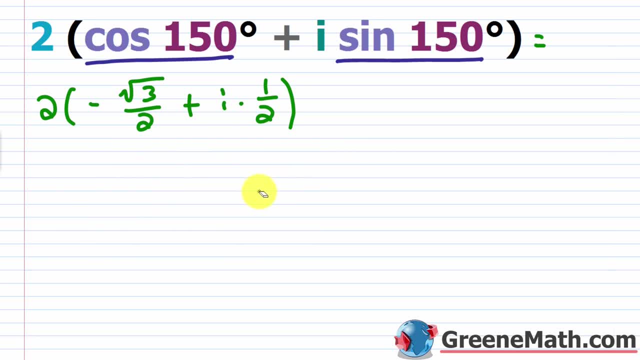 So let's just erase this. We don't need it anymore. And now I'm going to distribute the two to each term inside the parentheses. So I would have two times the negative of the square root of 3 over 2.. And then plus I'll do one half times two. 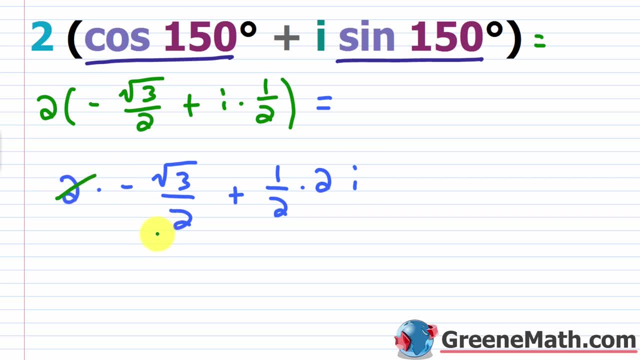 And then you could do times i OK. So basically we see that this would cancel with this and this would cancel with this, And in my rectangular form I have the negative of the square root of 3, basically plus one i, or you could just say plus i OK. 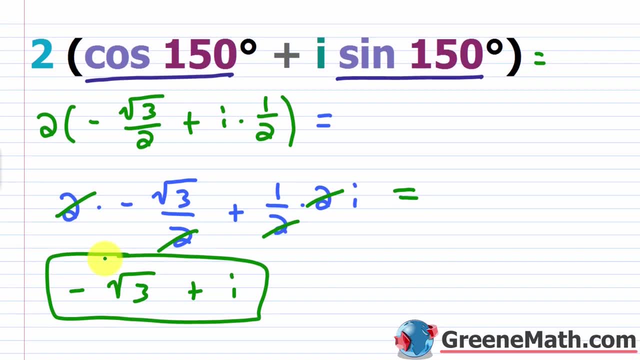 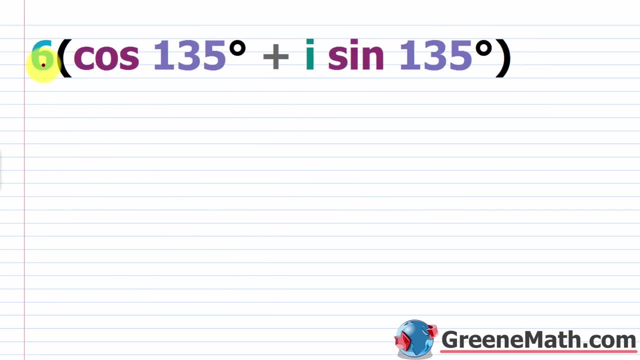 So this is my rectangular form, Or my standard form. And again, this right here is the polar form, where some people call this the trigonometric form. All right, let's look at another one. So we have the polar form here. 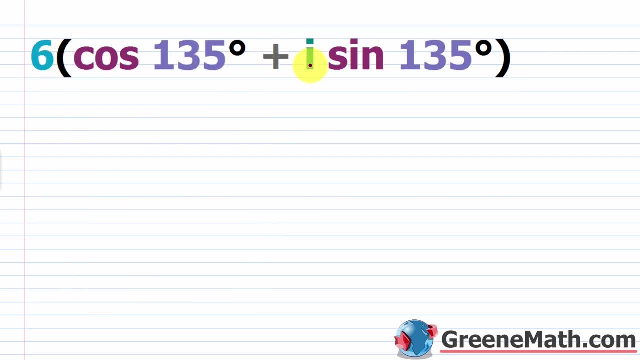 We have six times, You have the cosine of 135 degrees plus i times the sine of 135 degrees. So what is the cosine of 135 degrees? So again you're in quadrant two. so this is negative. What is the sine of 135 degrees? 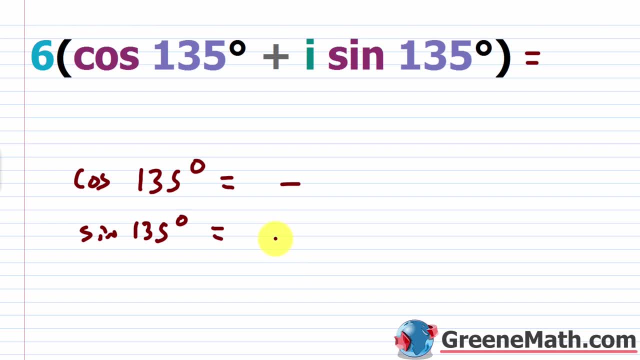 Again, you're in quadrant two, so this is positive. Remember 135 degrees: you have a 45 degree reference angle, So in each case, you're going to have square root of two over two, right? This guy is just going to be negative. 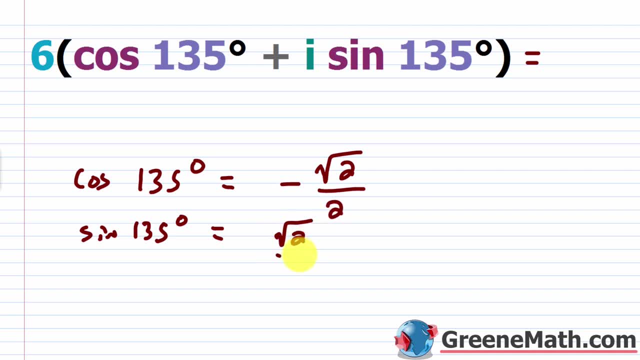 because cosine again is negative in quadrant two And this guy would be positive. OK. So basically I could replace this and say: I have six times This is going to be the negative of the square root of two over two, And then plus i times you're going to have the square root of two over two, OK. 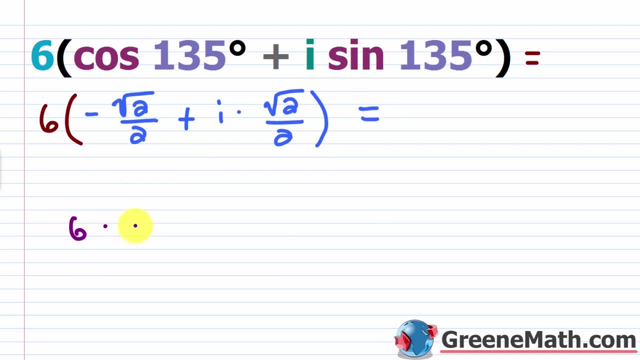 So if I distribute the six into each term, I would have six times the negative of the square root of two over two plus i times. Let me go ahead and switch the order here, So this makes more sense. We'd have the square root of two over two times six and times i. 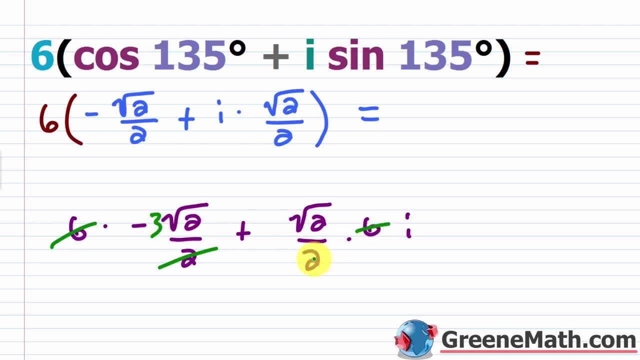 And I'll just go ahead and cancel this. This cancel with this and gives me a three. This cancels this and gives me a three. So basically, I'm going to have the negative of three times the square root of two and then, plus, you'll have three times the square root of two and then times i. 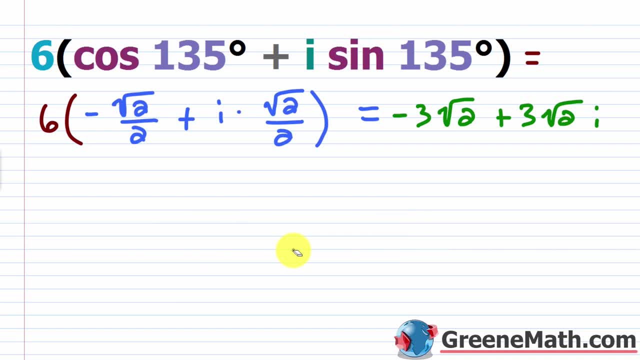 Now again a lot of times for clarity. you're going to move this around. Let me drag this down here, so it's a little bit better, so you can see things. I'll erase that and put that back And instead of having the i here, most books will do three. i like this. 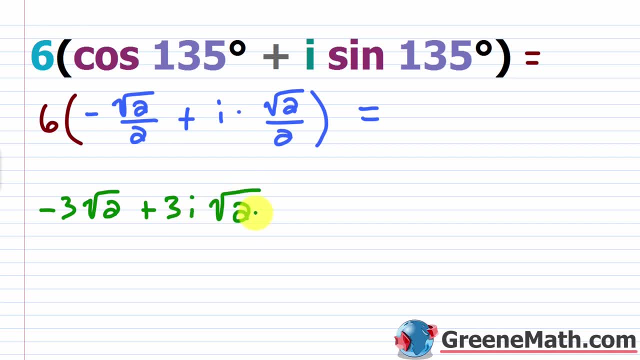 then times the square root of two. This is just to make it completely clear that the i is not under the square root symbol. OK, so the rectangular form here, or again the standard form, is negative three times square root of two plus three i times. 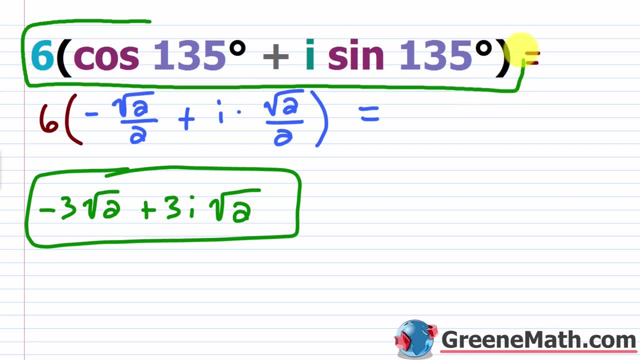 square root of two, And then again your polar form, or the trigonometric form, is going to be six times this quantity, cosine of 135 degrees plus i times sine of 135 degrees. All right, let's look at something more tedious now. 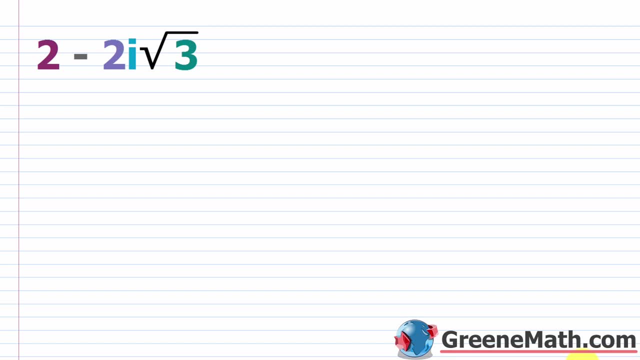 So we're going to convert from our rectangular form to the polar form. I'm going to give you three easy steps for this. The first thing that I always do is I figure out what quadrant my complex number is in. You can do that by just thinking about the real part and the imaginary part. 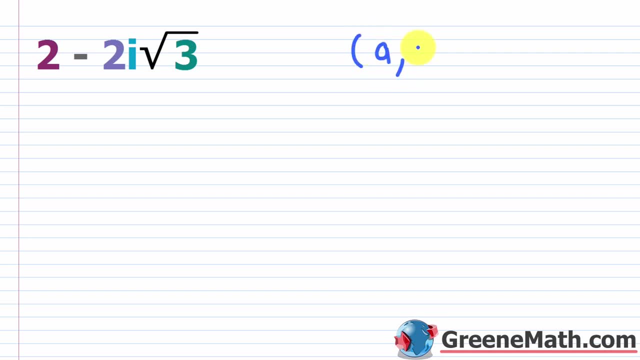 So, in other words, if you were to graph this again on the complex plane, it's a comma b. So if this is positive and this is positive, then you're in quadrant one. OK, if this is negative and this is positive, I'm going left and then up. so I'm in quadrant two. 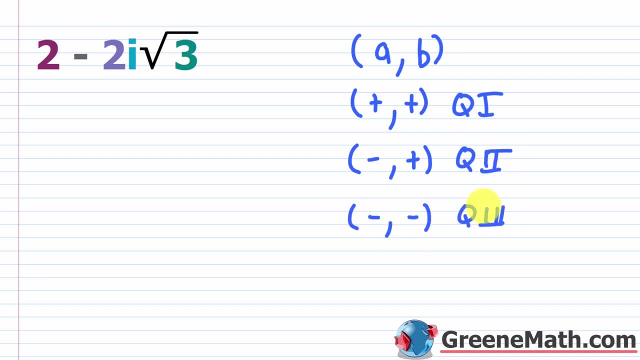 OK, if they're both negative, I'm in quadrant three, Right, I'm going left and then down. And then, lastly, if this is positive and this is negative, well, I'm going to be in quadrant four, right, because I'm going to the right and I'm going down. 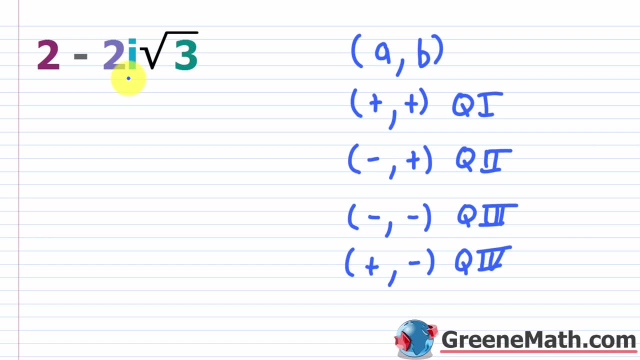 So just think about your real part and your imaginary part and ask yourself the question: If I was to graph this as a vector, OK, where would I be? Am I in quadrant one, two, three or four? OK, so that's the first thing you want to do. 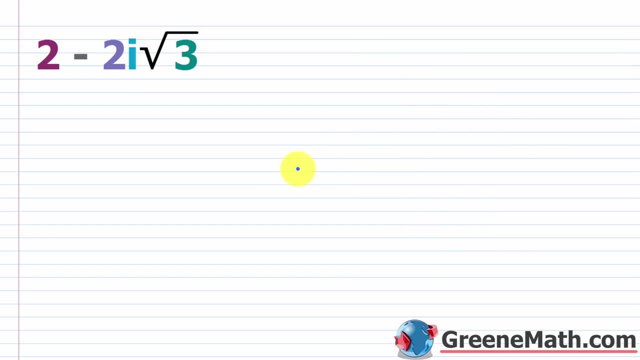 Now, if I look at this guy right here, I have two minus two i times square root of three. Again, this i is here for clarity. OK, if you want to, you can write this as two minus two times square root of three times i. 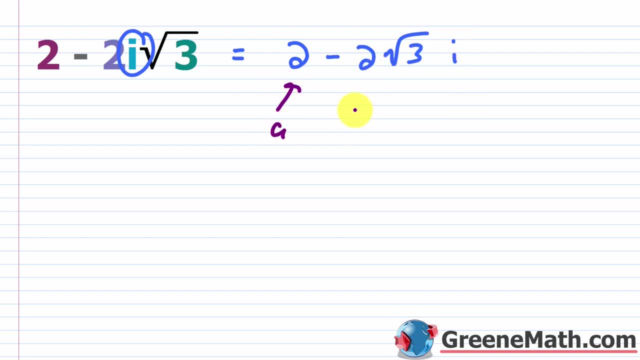 So it's crystal clear that this part right here is the real part and this part right here- you can go and take the negative with it- is the imaginary part, right? So a plus b i. OK, so we know that the real part is two, so that's positive. 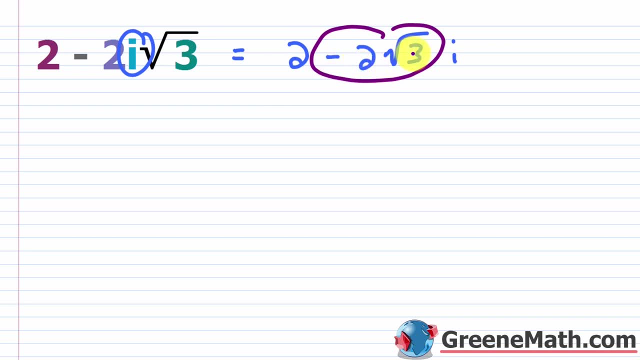 The imaginary part is negative. two times square root of three. That's negative. So I'm going to the right, OK, and then I'm going down. That means I'm going to be in quadrant four right, Because again, this is positive and this is negative. 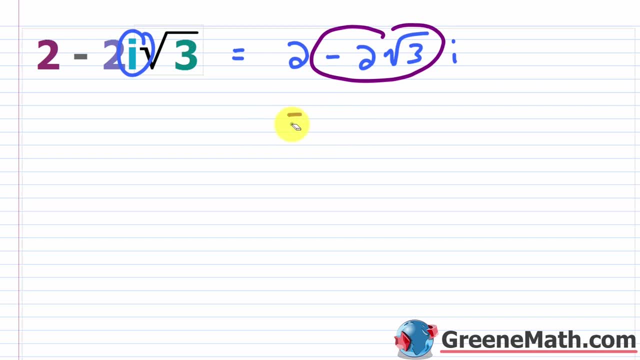 And you're thinking about this in terms of the complex plane. OK, so now I know that theta is in quadrant four. We need that for later on when we're getting our angle theta. So if we want to get this trigonometric form of the polar form, it's r times. 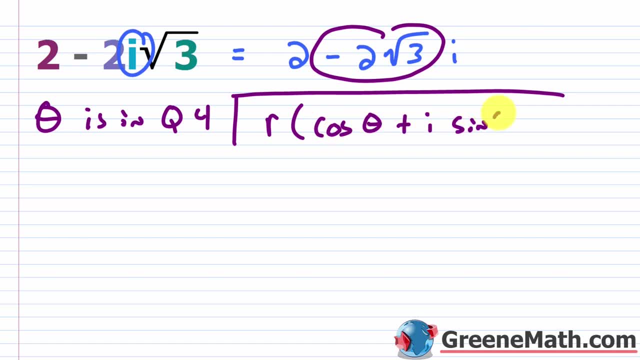 cosine of theta, plus i times the sine of theta. OK, that's all it is. So I need to figure out what r is, and I need to figure out what theta is, and I'm done. So how do I figure out what r is? 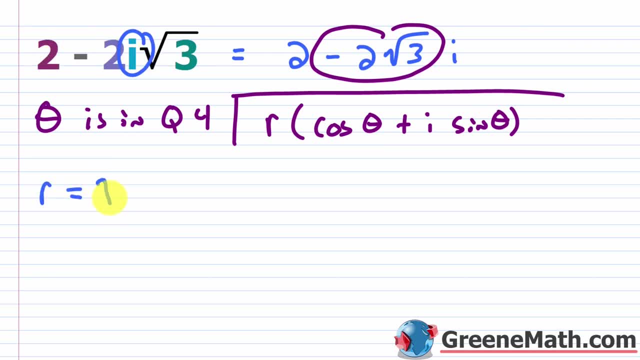 R again is just the absolute value of the complex number. OK, we've been doing this forever. It's the square root of the real part squared, So two squared plus the imaginary part Again. if you're writing it like this, 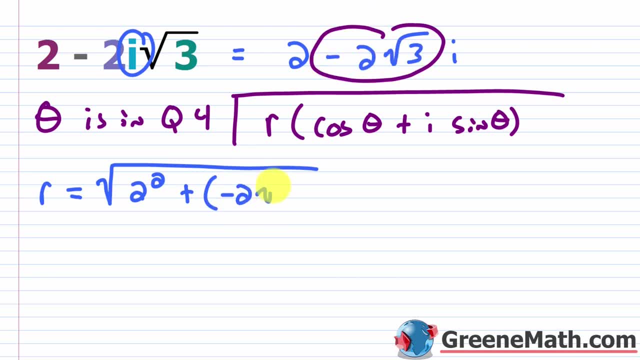 it's crystal clear: negative two times square root of three. So negative two times square root of three. OK, this guy being squared. Some students make a mistake when it's written like this. Again, they put i in there for some reason. 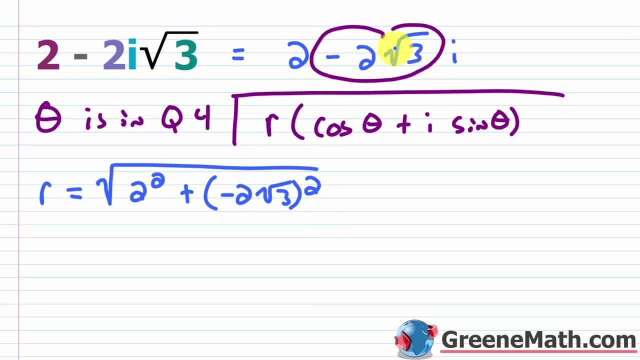 Again. just go ahead and write it like this, So it's crystal clear that this is the imaginary part. You want the a squared plus the b squared, or the x squared plus the y squared. whatever the notation is OK: the real part squared plus the imaginary part squared. 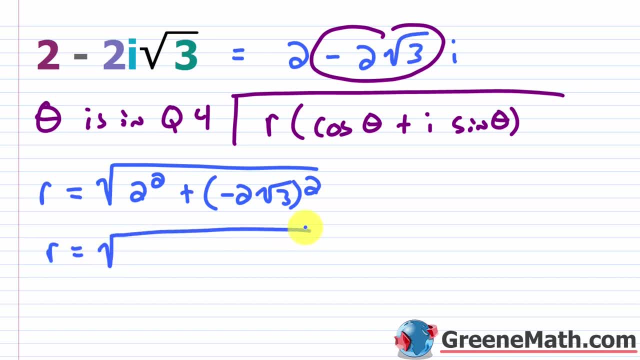 OK, that's what you want. So we have: r is equal to, the square root of this is four. And then basically, you have negative two squared, which is four, and you have square root of three squared, which is three. So four times three is twelve. 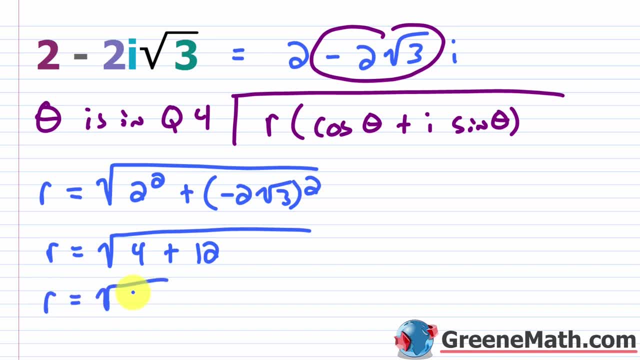 So I put plus twelve here. OK, so r is equal to the square root of 16.. So r is equal to four. OK, so the first part of that, OK, the first part of that is done. So r is equal to four. 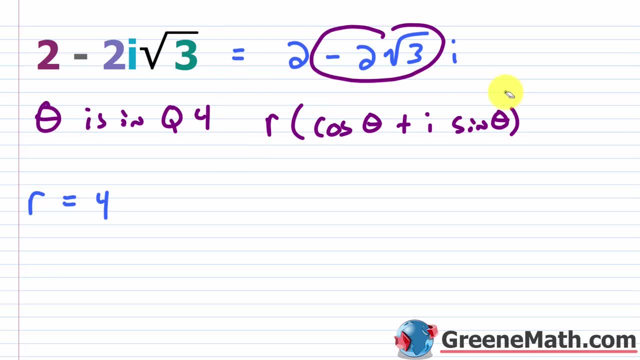 And this looks like I made a radical here. I was just making a border, So let me kind of clarify that and put this maybe like this or something. That would be better, I think, And maybe I could just do it upside down. 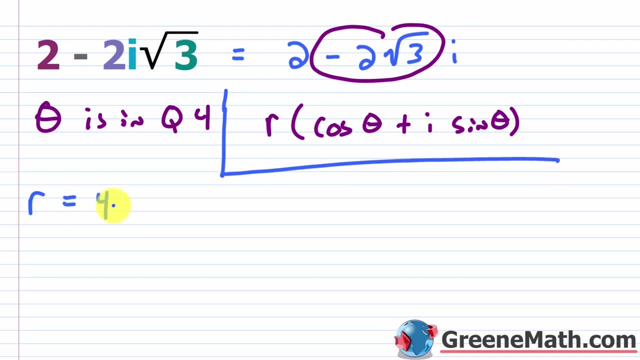 I'm just trying to make a border. That's not a radical. So r equals four, OK, so now I need to find theta. So what is that going to be? Again, you use the fact that the tangent of theta is y or the imaginary part. 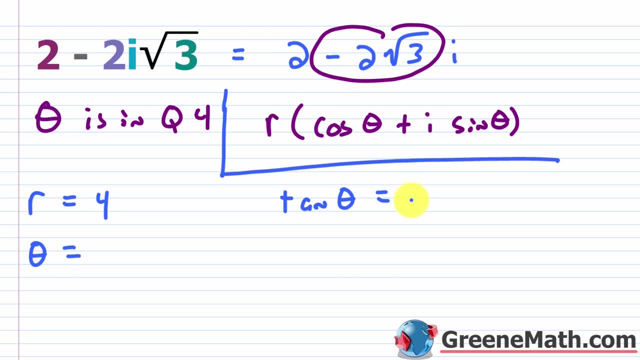 over x or the real part. OK, so the imaginary part. You have your negative two times square root of three over your real part, which is two. OK, so you can go ahead and cancel this with this, And this is the negative of the square root of three. 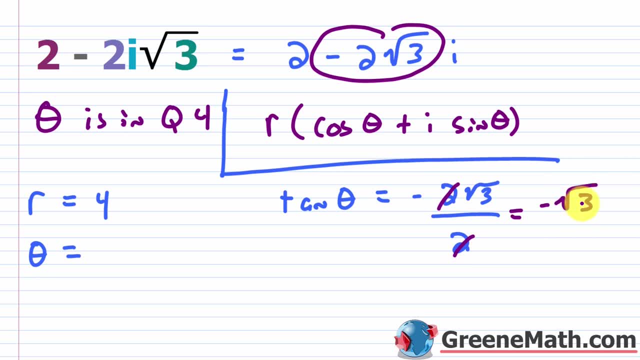 OK. now what I would do, OK- is not punch this into the calculator as the tangent inverse of negative square root of three, because you're going to get something in quadrant four rotating clockwise. Now your teacher may allow that as an answer. 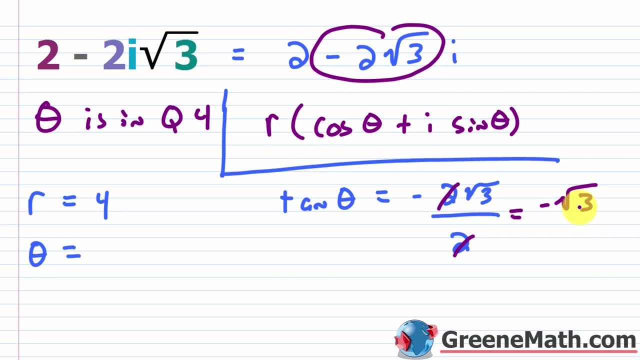 But typically you want something between zero and two pi, where zero is included, And the two pi is not OK. so what I'm going to do is I'm going to say that I want the tangent inverse of the square root of three, And this is going to give me 60 degrees. 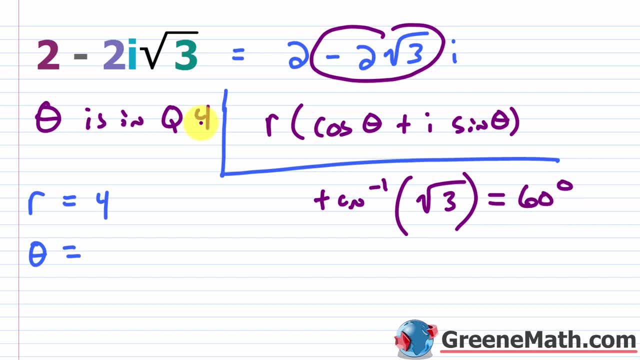 OK, this is going to be my reference angle and I'm going to be in quadrant four. OK, remember, we figured out we're in quadrant four for this reason, So in quadrant four. if I had an angle, with a reference angle of 60 degrees, to find that I would do 360 degrees minus 60 degrees, which gives me. 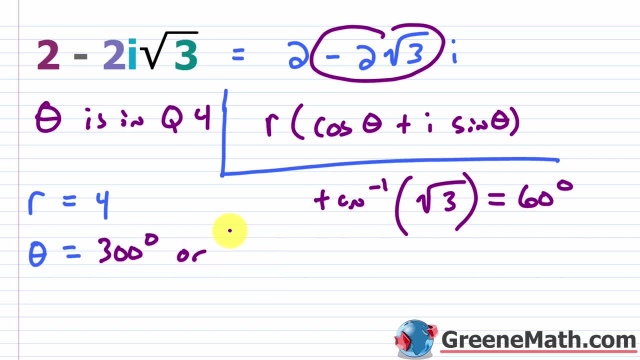 300 degrees, Or in terms of radians it would be five pi over three. So now that we've done all this work, OK, we are ready to write this guy in polar form, And I guess you can get rid of this. 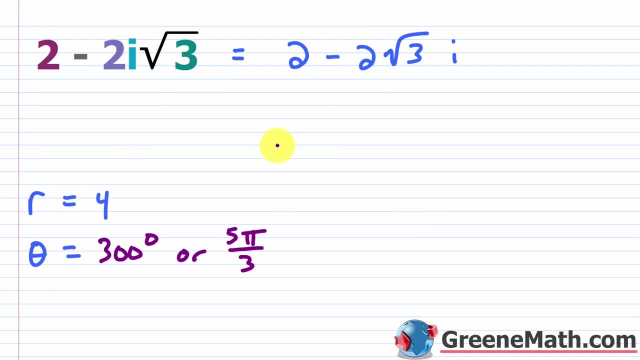 We don't really need it anymore. I'm just going to write this and say that basically this guy- and I'll just even erase this- would be the R, which is four times you would have cosine of your angle. So you can use either one you want. 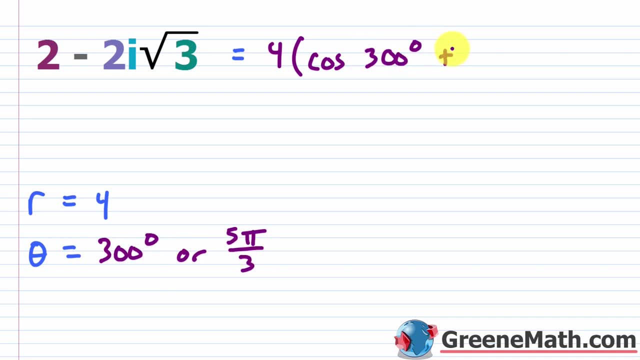 You can do it in radians or degrees. So 300 degrees And plus again. I'm going to put I first and then times your sine. OK, of that same angle, 300 degrees. If you want to write this with radians, all it is, I'll put equals again. 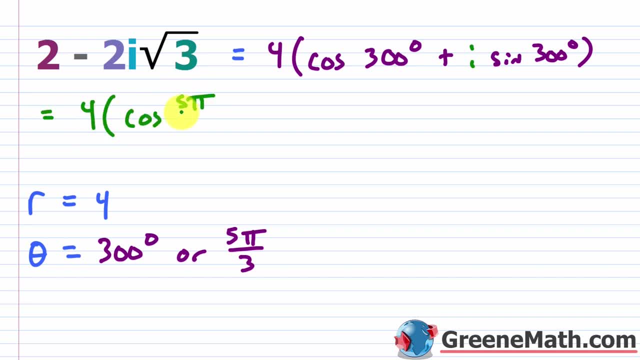 So four times you're going to do cosine of five pi over three, OK, and then plus I times the sine of five pi over three. So always go with what your teacher says. If they want radians or degrees, just ask them, OK. so we basically have this done. 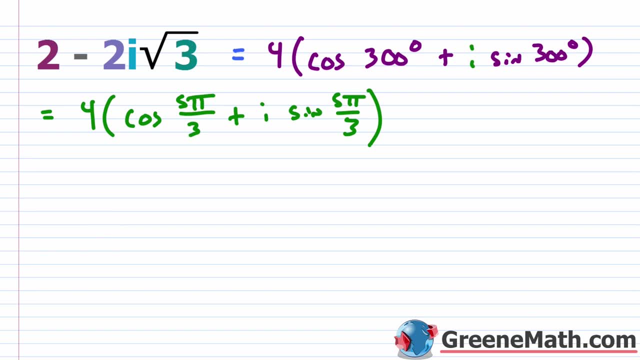 And also, if you wanted, you can use that little abbreviation. Let me just show you that real quick You could do. this is four times CIS. So again the C, the I and the S. that's where the abbreviation is coming from. 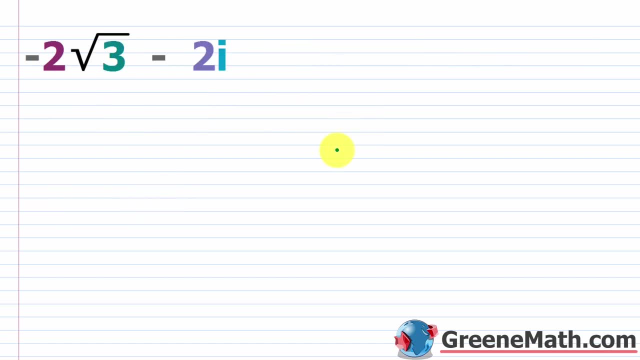 And then times. let's just go and say five pi over three. Let's look at another example. So we have negative two times square root of three minus two I. So again, the first thing you want to do is figure out what quadrant is theta going to be in. 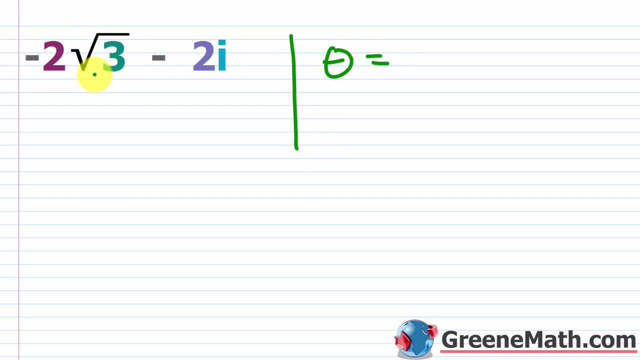 Again, you can speed this up at this point. Again, here's the real part: It's going to be negative. Here's the imaginary part. It's going to be negative as well. In other words, if you were to graph this: 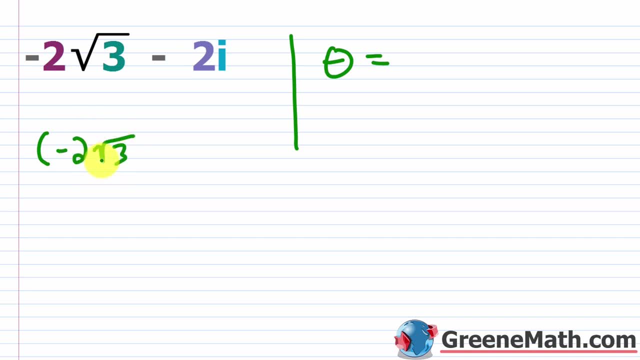 you would have negative two times square root of three. This would be your location on the real axis, And then you would have negative two. That'd be your location on the imaginary axis. So, in other words, this is negative and this is negative. 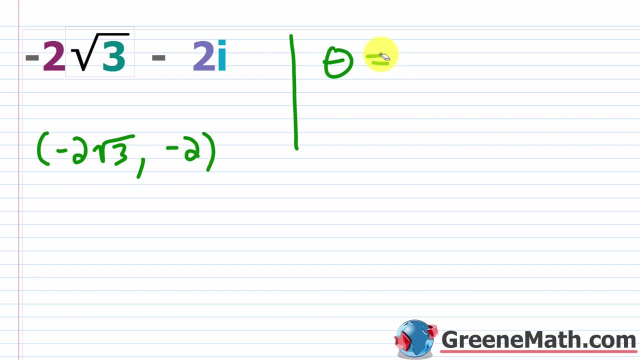 So I know I'm going to the left and down, So I'm going to be in quadrant three and I put equals here. I should just put: is in quadrant three. OK, so we can keep that straight. Now what I want to do is quickly find my value for R. 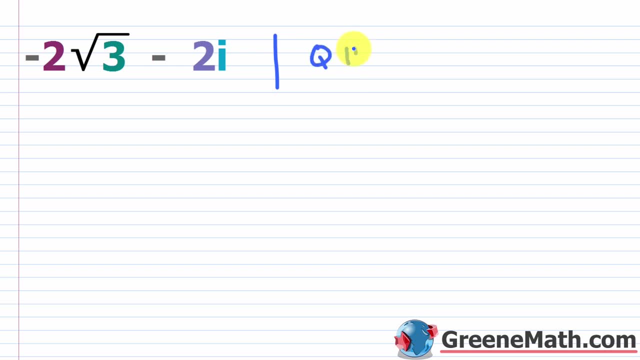 I'm just going to make that a little bit more clean. So my quadrant three, I'll just put for my angle theta. So for R, again, it's the absolute value of this complex number. However you remember it, remember, it's the square root of the real part. 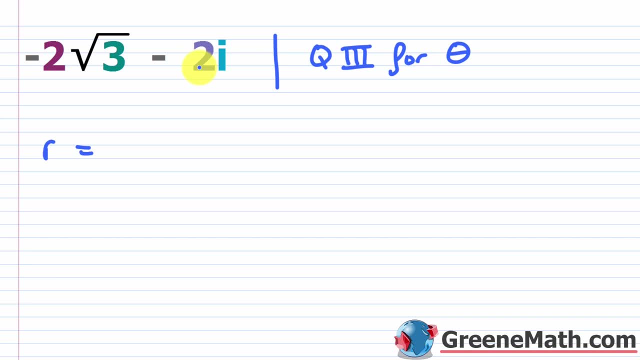 squared, plus the imaginary part squared. however, they're giving that to you, OK, so I'm going to take the square root of I'll take negative two times a square to three being squared, and plus I'll have my negative two being squared. OK, so from here I know that basically negative two squared is. 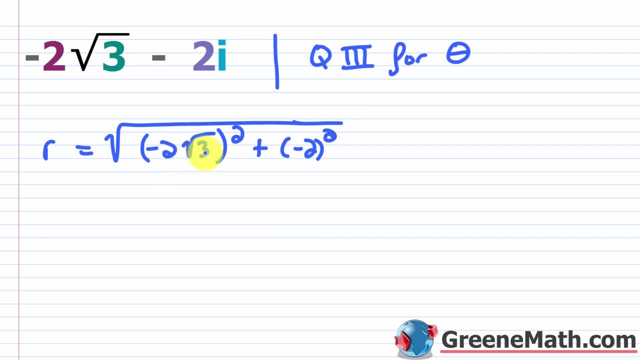 four square to three squared is three. So four times three would be twelve, And again, we already know this. So this is going to end up being four, right, Because this is twelve plus four, That's going to be sixteen. Square to sixteen is four, right. 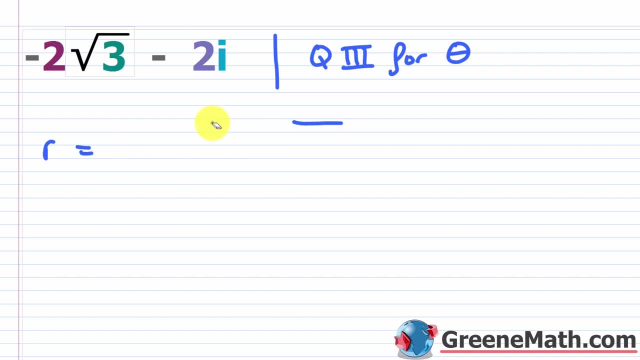 But to go through the steps, this would be four. Again, twelve plus four is sixteen. Square to sixteen is going to be four. So R is four. We know that. So let's find theta. This is the one that takes a little bit longer. 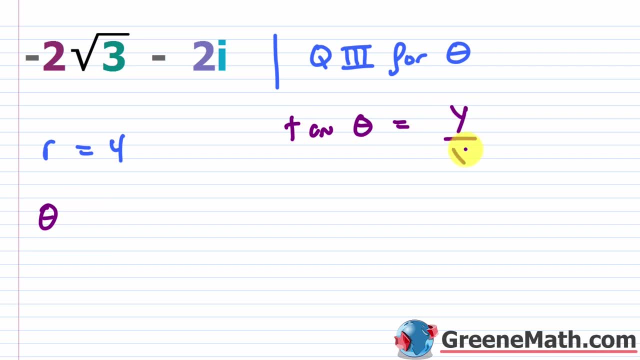 So we know that tangent of theta again is Y over X, where you could say B over A. If you think about this in terms of the traditional way we think about complex numbers, it's going to be the imaginary part over the real part. 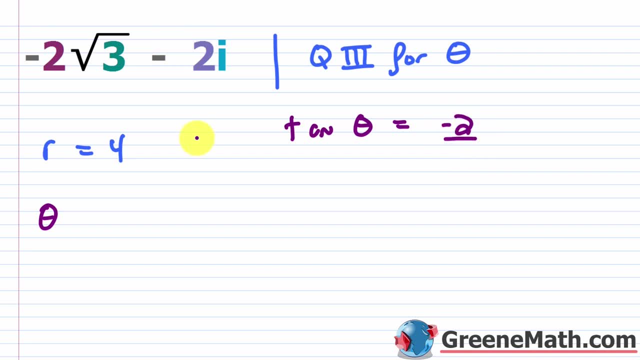 So the imaginary part is negative two, so negative two, And the real part is negative two times square root of three. OK, so this is going to cancel and I'll have one over the square root of three, If I rationalize the denominator there, so times the square root of three. 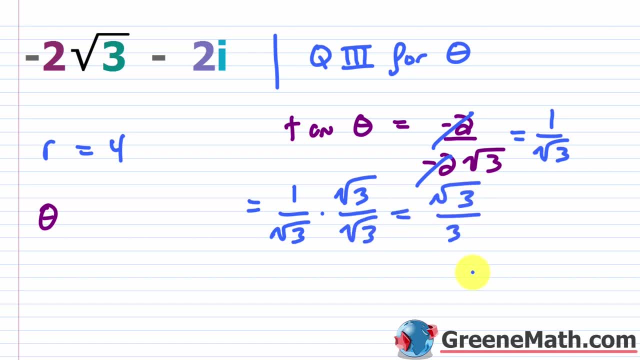 over the square root of three. this is the square root of three over three. OK, so basically, if I punched up the inverse tangent of square root of three over three, I'm going to get something in quadrant one. Remember, I'm looking for something in quadrant three. 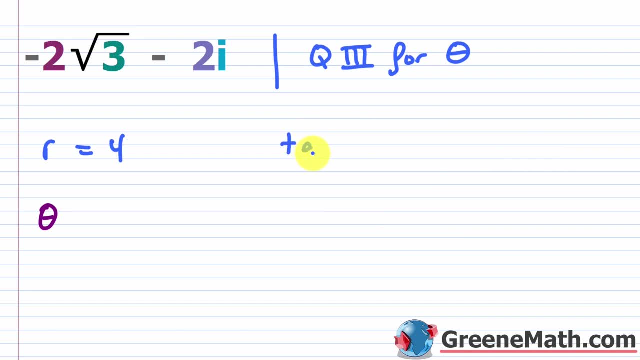 OK, so let's go and set the sum. I want to go inverse tangent, OK, inverse tangent of square root of three over three, like this. So you hit that up on your calculator, You're going to get 30 degrees, OK, and again in quadrant three. 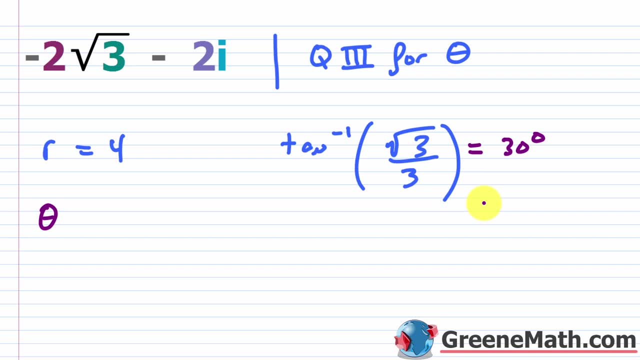 if I have an angle, with a reference angle of 30 degrees, to find that I would do 180 degrees plus 30 degrees OK, which would give me 210 degrees. So theta is going to be 210 degrees. So now that we have all the required information, I can just put equals. 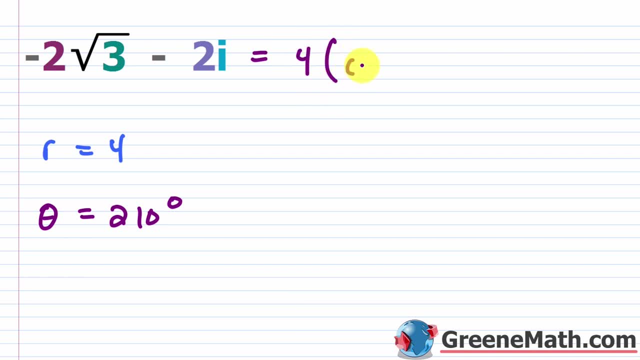 I'm going to take my R value, which is four, and I'm going to multiply by again. You have your cosine of this angle: 210 degrees, plus I times the sine of this angle, which is 210 degrees. So that's basically it. 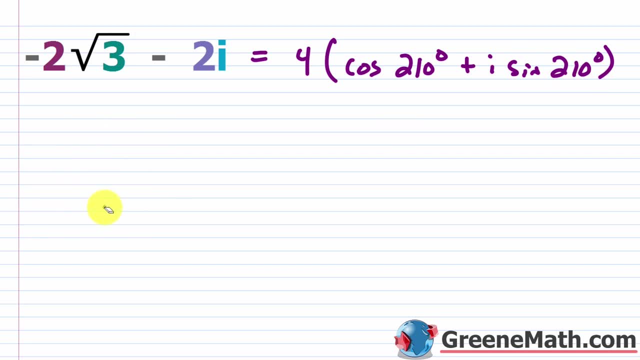 That's your polar form. Now if you want to write this with radians or write it as an abbreviation, you can keep putting equals. So 210 degrees in terms of radians would be seven pi over six. So you could say this is four times you'd. 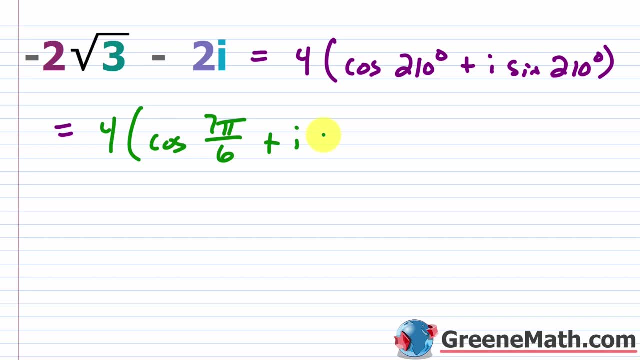 have the cosine of seven pi over six, plus I times the sine of seven pi over six. And again one more time: this C, this I and this S. you can use it to abbreviate, So you could say: this is four and you go. 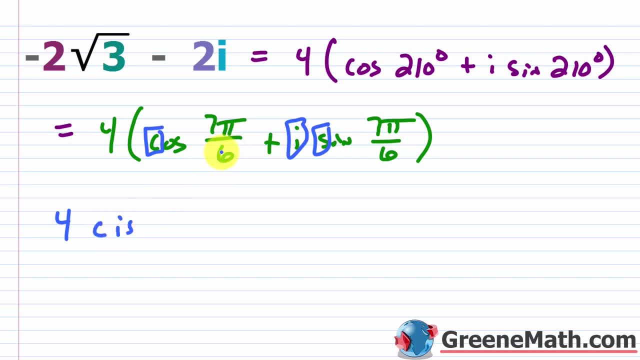 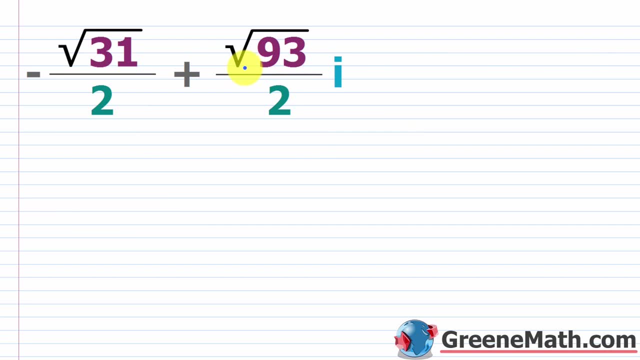 CIS or CIS, and then you'll say your angle. So again you could do degrees or radians, whatever We'll do seven pi over six. So another way to write it. this is the shorthand. All right, let's look at one more example. 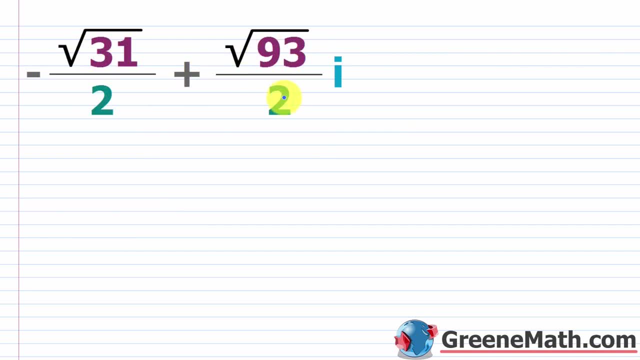 So we have the negative Negative of the square root of thirty one over two, plus the square root of ninety three over two times. I Again, just be careful- Sometimes I'll put the I up here because you're working with a radical- Just be able to separate the imaginary part from the real part. 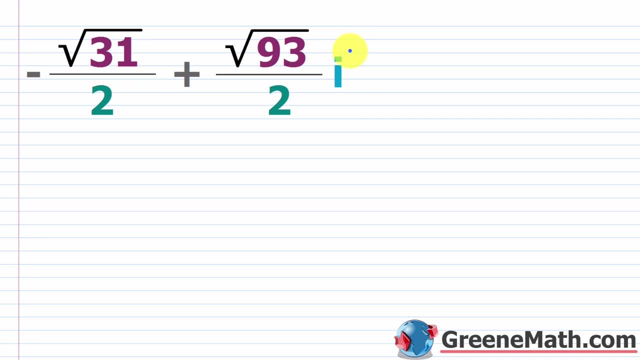 OK, you need to know what those are and you need to not get I mixed into that, OK, so what I'm going to do here again is think about what quadrant am I going to be in? OK, this is negative, This is positive. 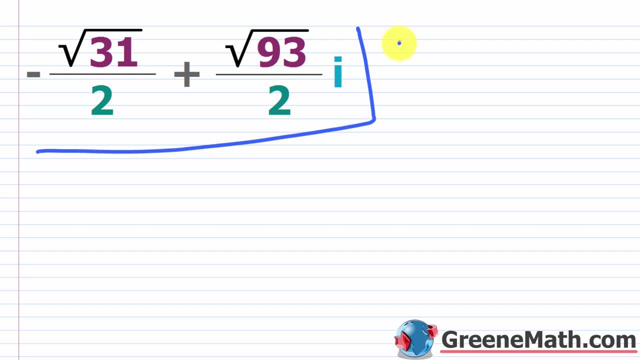 So I'm going to the left and I'm going up Right, So I'm in quadrant two. So theta is in quadrant two. OK, very important to understand where I am. Now. once I understand that, I'm in quadrant two again when I go to find theta. 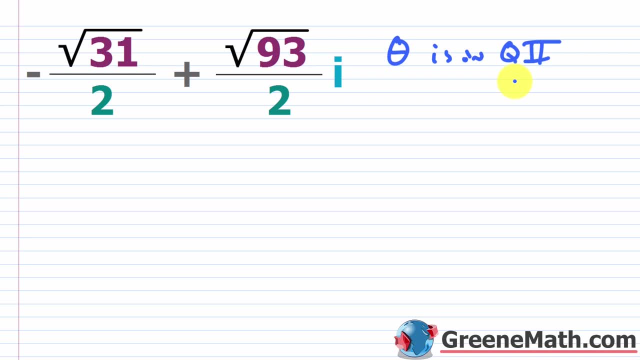 OK, I'm going to basically get a reference angle and then use that in quadrant two. Well, let's find R first, because it's a little bit easier. So R equals again the square root of take your real part being squared So negative of square to thirty one over two. 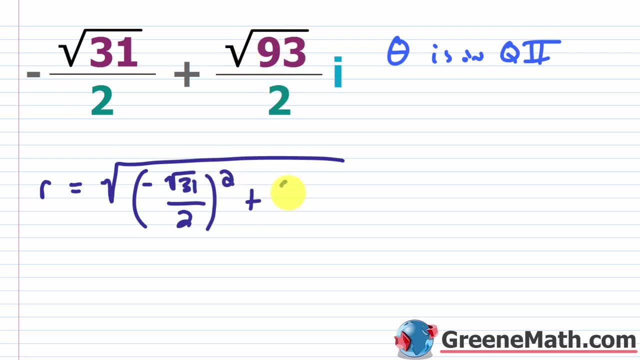 We're going to square that, plus take this guy, the imaginary part, so the square root of ninety three over to this guy squared. OK, so R is equal to what? If I square this, I'm going to get thirty one over four. 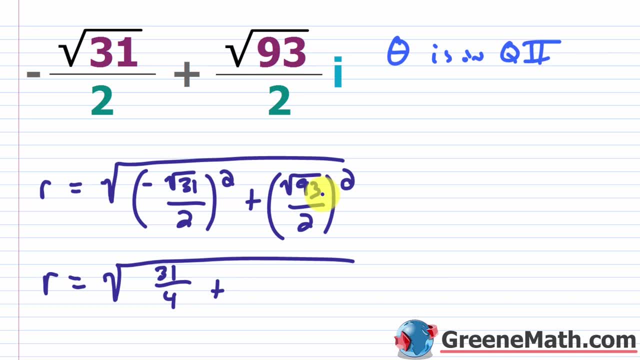 So the square root of you'll have thirty one over four. plus this guy would be ninety three over four. OK, if you add those together you're going to get one hundred twenty four over four. So one hundred twenty four over four. If you make that division you're going to get thirty one. 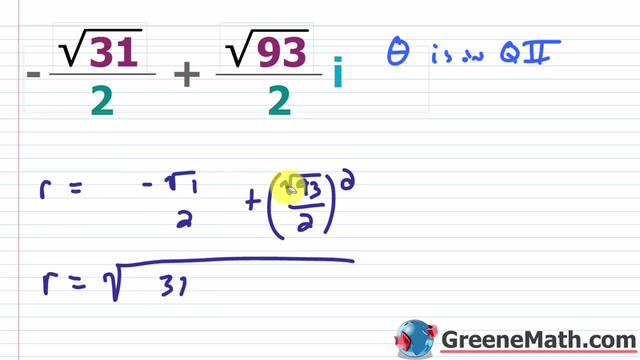 OK, you can't simplify that. Thirty one is a prime number. So basically, R is just the square root of thirty one. OK, so R is equal to the square root of thirty one. OK, let's work with theta. So the tangent of theta is what? 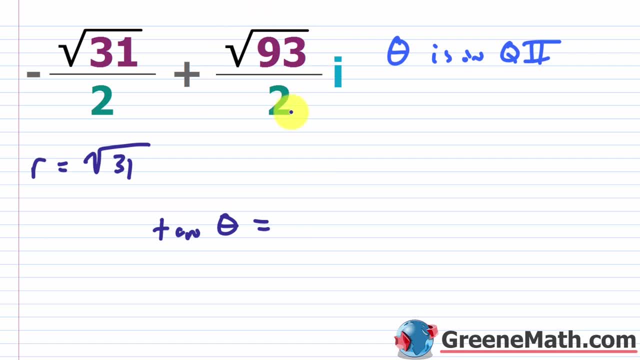 It's the imaginary part, or Y or B, however you want to think about it. So square root of ninety three over two, over the real part, which is X or basically A, however you want to think about that. I'm just going to flip this guy because 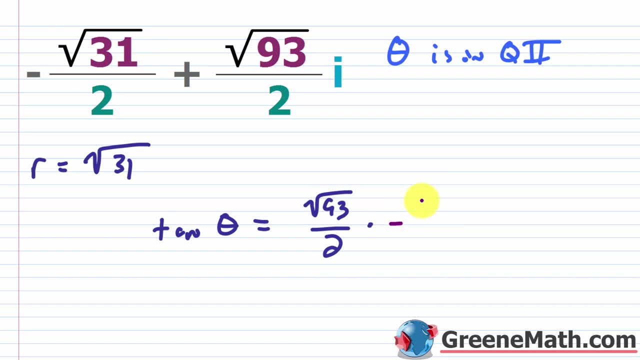 when you divide fractions, you multiply by the reciprocal, So I'll put the negative of two over the square root of thirty one. That's going to allow me to cancel this with this. I know that from the quotient of four radicals I can divide here. 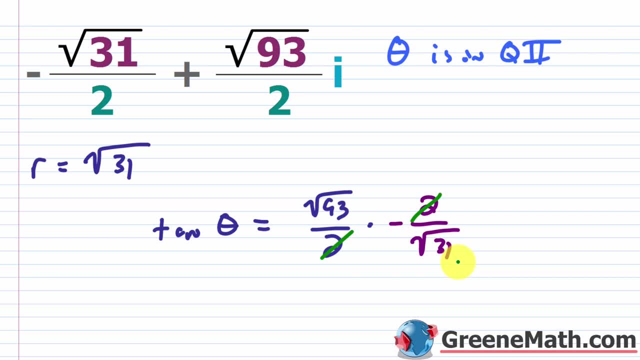 So ninety three divided by thirty one is three. So I can basically say this is the negative- OK, the negative- of the square root of three. Now we know from the first example, this guy is going to have a reference angle of 60 degrees. if I did the inverse tangent of square root of three. 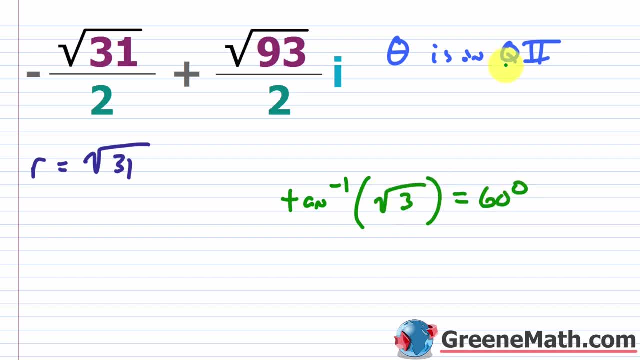 I'm going to get 60 degrees. So, because I'm in quadrant two, what I want to do is I want to take one hundred eighty degrees and I want to subtract the reference angle of 60 degrees And that's going to get me to one. 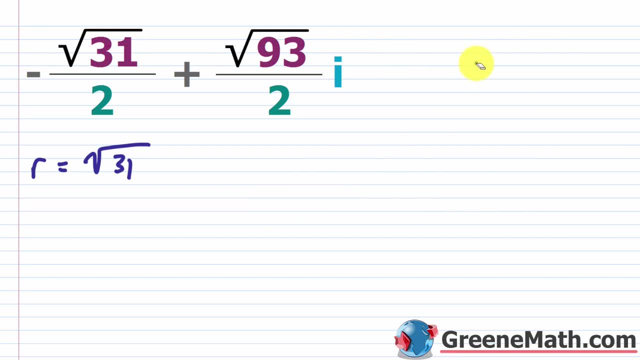 hundred twenty degrees. So theta is one hundred twenty degrees here. OK, so theta, theta is one hundred twenty degrees. Or in terms of radians you could say this is two pi over three. OK, so basically I'm ready to set this up. 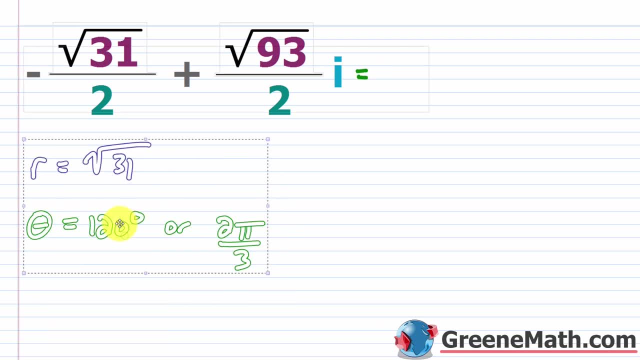 I can go ahead and say this: equals- and let me just drag this out of the way, Put this down here. I'll say my R value, which is the square of thirty one times. Let's just go and use degrees first. I'll say cosine of one hundred twenty degrees plus I times. 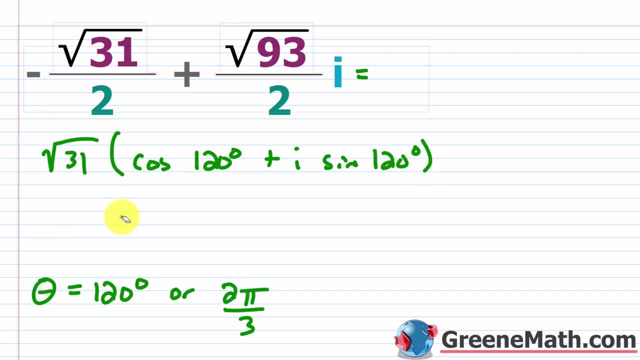 The sine of one hundred twenty degrees. OK, And again you can keep going, Right? So if you want to put this in terms of radians, I'll put equals, I'll do square root of thirty one times the cosine of two pi over three, and then plus I times will do the sine of two pi over three. 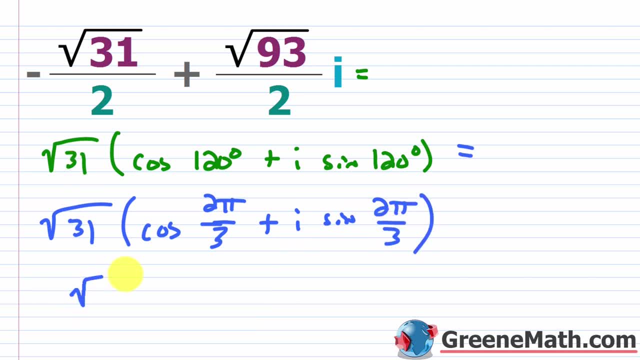 OK, like this. And lastly, if you want to do your abbreviation, take your R value, which is square to thirty one, and then times that CIS, or the CIS again, the C, the I and the S, So CIS. That's how you can remember that. 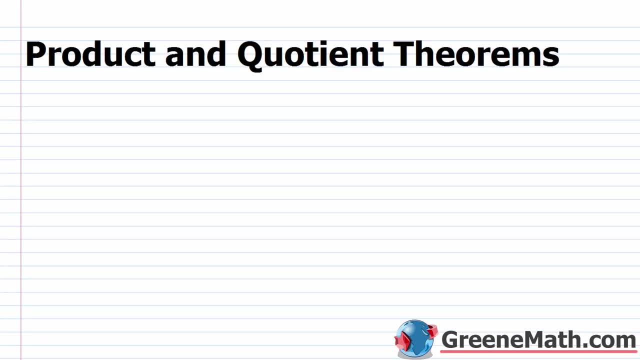 And then times your one hundred twenty degrees. In this lesson we want to talk about the product and quotient theorems. All right, So in the last lesson we talked about how to write a complex number and what we call the trigonometric. 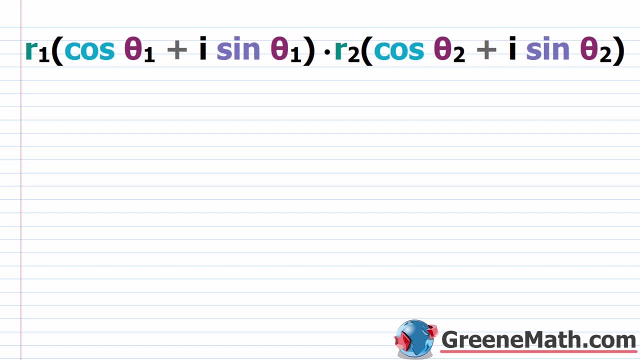 form. Most people call this the polar form, And here what we want to do is learn how to quickly multiply or divide two numbers, if they're in polar form, using something called the product or also the quotient theorems. OK, so I'm going to start off with the product theorem. 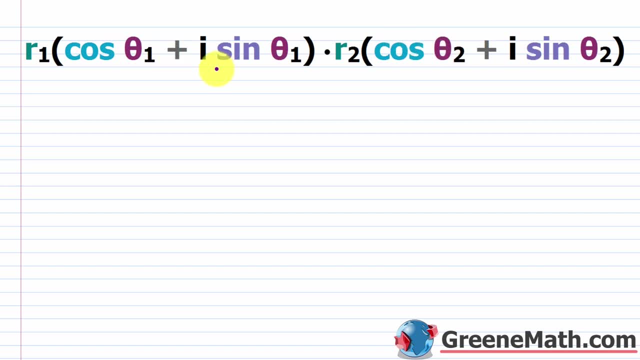 And basically we have these two generic, complex numbers written in polar form. Right, Remember, when you think about the R value, if it's as a vector, if you think about it that way, this is the magnitude or the length of the vector. 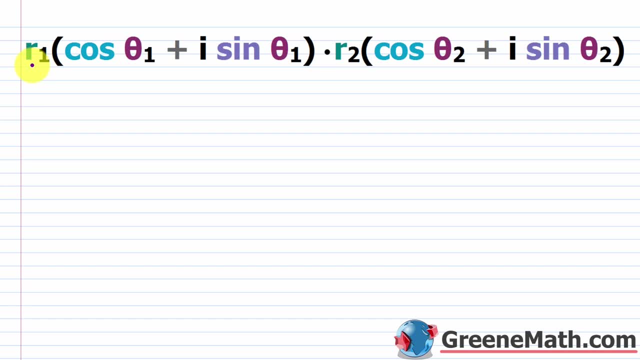 Or you could also think about it as the absolute value of the complex number. OK, so that's the R value in each case. When you think about theta- OK, this is going to be. if you think about this as a vector, it's the direction angle. OK, 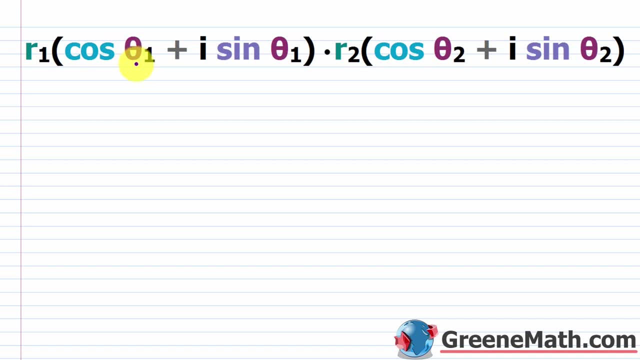 Or, if you think about it here, a lot of books will also call this the argument. OK, so you hear that terminology. So here we have this: R sub one times the quantity, cosine of theta sub one, plus I times sine of theta sub one. 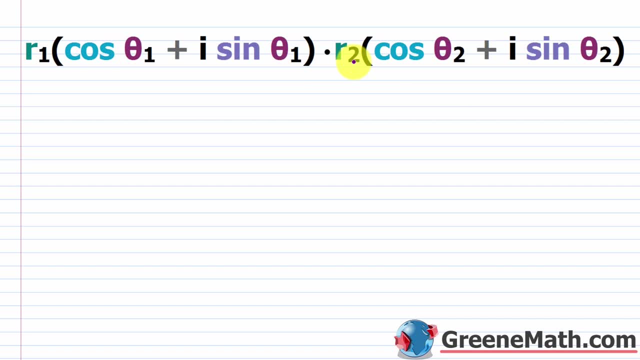 OK, then times with this other complex number, so R sub two multiplied by the quantity cosine of theta sub two, plus I times the sine of theta sub two. OK, so all I need to do to derive my little product theorem, OK, is just use some foil. 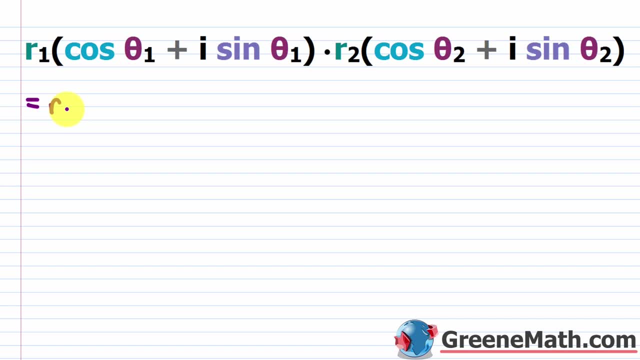 So I'm going to start out by multiplying R sub one times R sub two, So R sub one times R sub two. Then I'm just going to set up some brackets here and I'm going to put these two inside. So I'm going to go the cosine of theta. 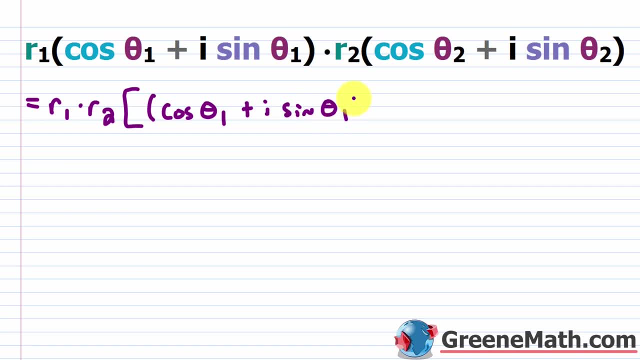 sub one, plus I times the sine of theta sub one, And then I'm going to go cosine of theta sub two, and then plus I times the sine of theta sub two. OK, so all we're going to be doing is foil. Nothing fancy here. 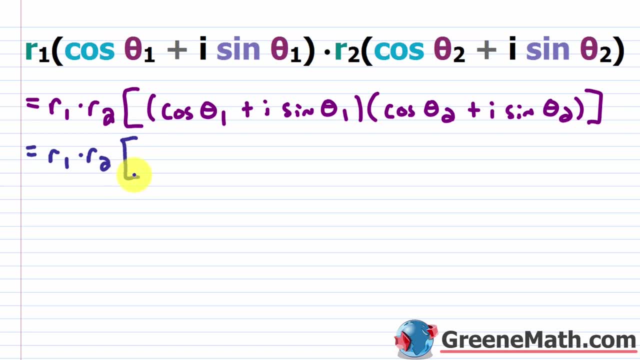 So I'm going to put equals R sub one times R sub two, And then let me open up these brackets And if we're doing foil, we're going to do the first term. So this guy times this guy. So this would be my cosine of theta sub one. 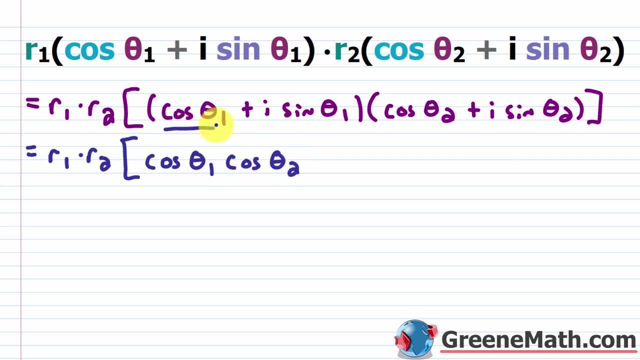 Times the cosine of theta sub two. Then I want to do my outer. So this one times this one, Let me go and put plus, I have an eye there. Let me put that out in front and then I'll just do my cosine of theta sub one times my sine of theta sub two. 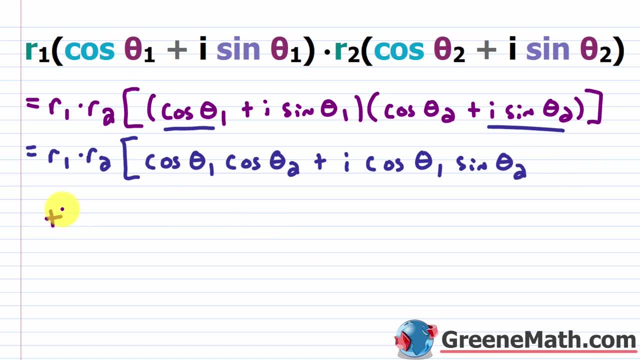 OK, I'm going to put this down here because it's going to run off. So I'm going to put plus and I'm going to erase this and this, And now we're doing the inside Right. So it's basically going to be: let me change the color. 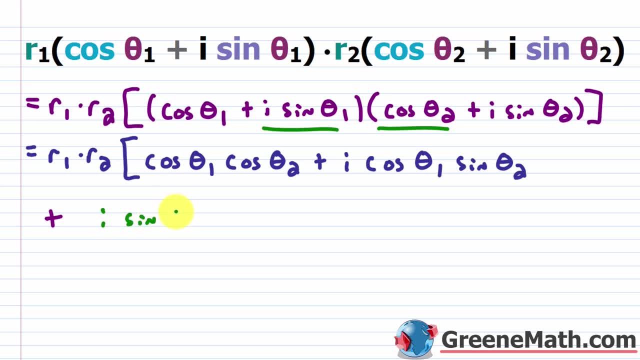 This one times this one. So you would have: I times the sine of theta sub one Times the cosine of theta sub two. OK, And then, lastly, we have the L Right. So this guy times this guy, I times I is I squared. 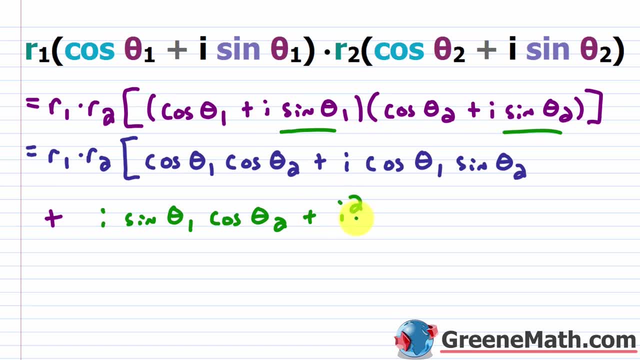 Now you can put plus I squared, But remember this is negative one by definition, So we're going to change this in a moment. Then you have your sine of theta sub one times your sine of theta sub two. OK, let me close the brackets there. 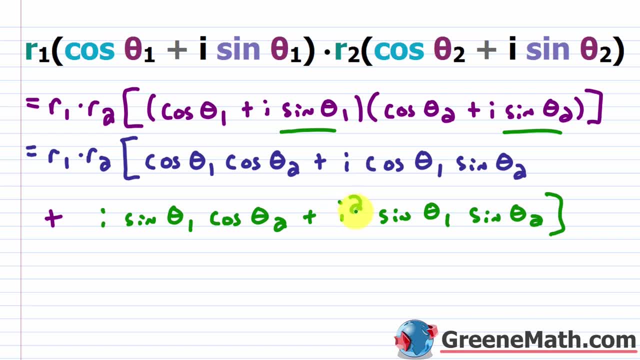 because this is being multiplied by all of those. Now, as I just said, I squared is negative one, So we can erase this and just put a negative sine here. OK, And now what I want to do is I want to group everything where the terms that have 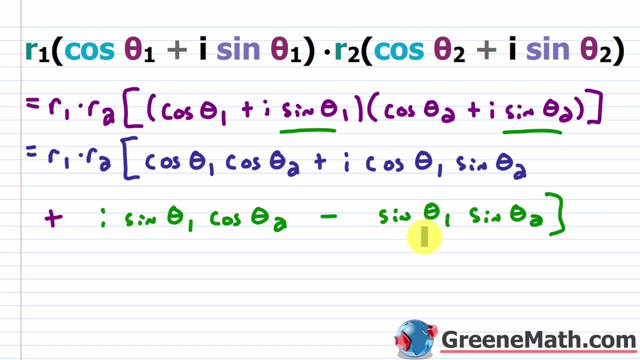 an I are next to each other and the terms that don't have an I are next to each other. So I want this one and this one to be next to each other. And then let me change my highlighter color here. I want this one and this one to be next to each other. 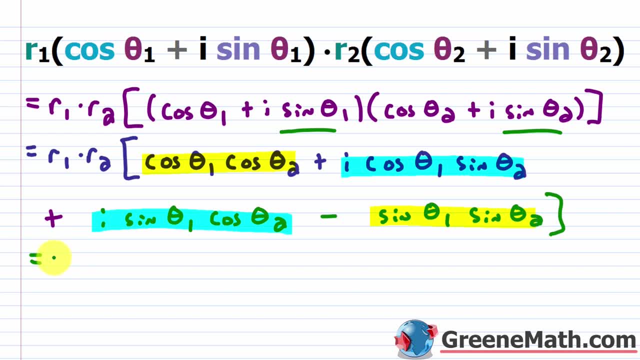 OK, so let me go ahead and do that real quick. I'm going to put equals R sub one times R sub two, And then inside the brackets here I'll go cosine of theta sub one times cosine of theta sub two, And then I'm going to do minus. 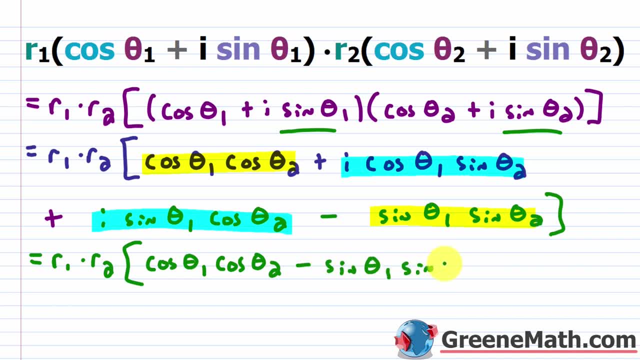 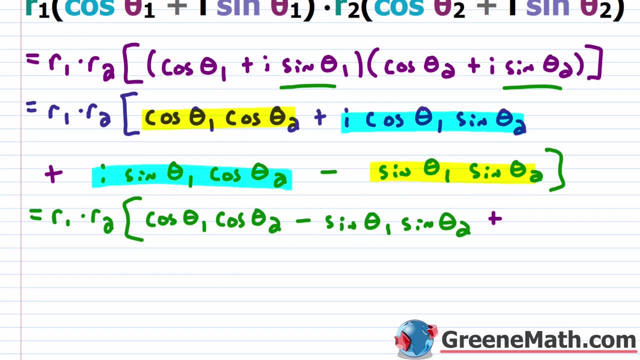 I'm going to go sine of theta sub one times sine of theta sub two. OK, and then we'll go ahead and say plus- Let me scroll down and get a little bit of room here- I'll say I times the cosine of theta sub one times the sine of theta sub two. 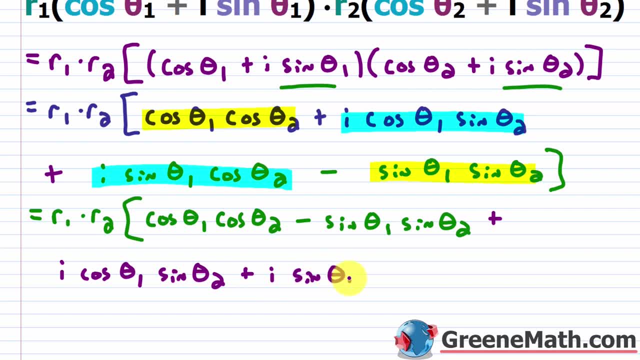 And then I want to put plus. I have my I times the sine of theta sub one times the cosine of theta sub two. OK, so let me close the brackets there Now. the reason we group these guys together is because to further simplify this, or to get into the form you're going to see in your book. 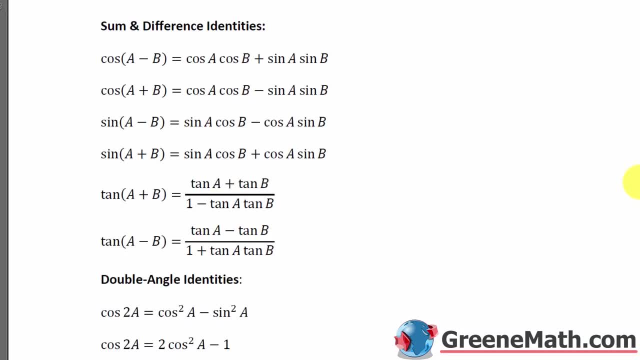 you're going to use an identity. So if we go back to our little handout and we go to the sum and difference identities, I want to call your attention to this first one. So we have the cosine of some angle A plus some angle B. 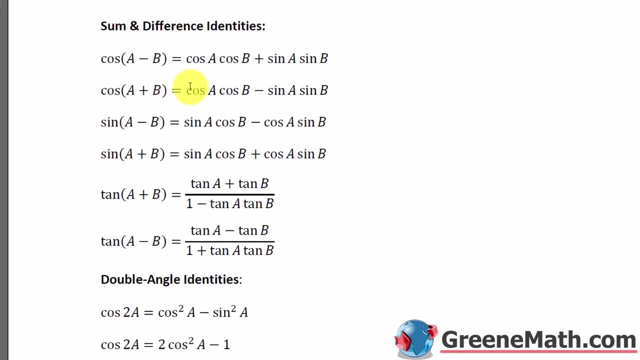 OK, in our case it's theta sub one and theta sub two. OK, so the cosine of A times the cosine of B, minus the sine of A times the sine of B. OK, so what we have is this guy on the right. 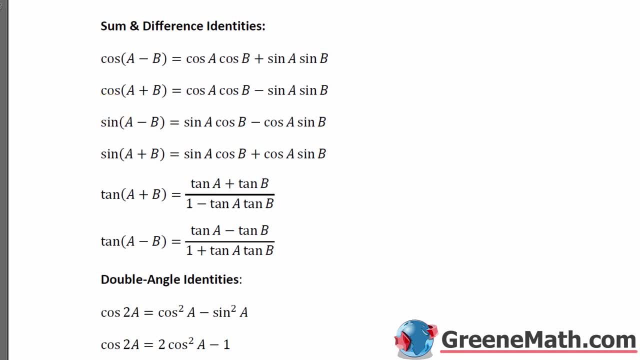 We want to transform it to what it shows on the left? OK, that's perfectly legal. So what we're going to do is say the cosine of theta sub one times the cosine of theta sub two, So it's just like having A and B, OK. 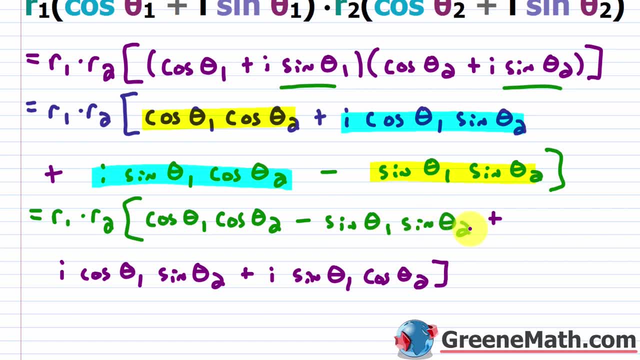 minus the sine of theta sub one times the sine of theta sub two. Well, we could write that as the cosine of: we'll have the theta sub one plus the theta sub two. OK, so I'm just using that identity to make this more compact. 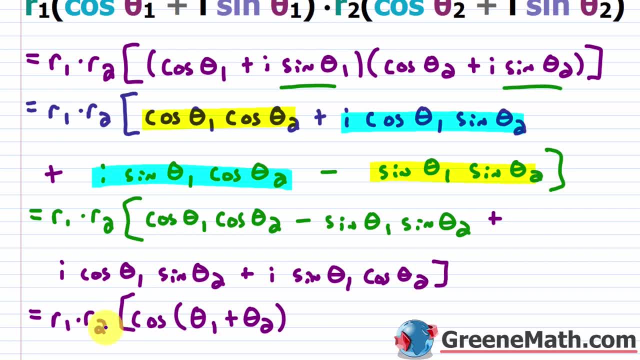 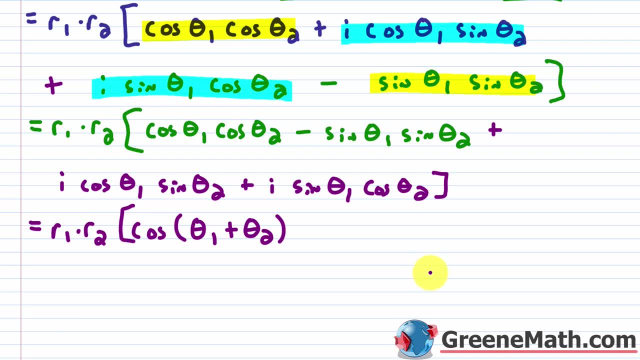 So let me put my bracket there, Let me put my R sub one times my R sub two, Let me scroll down Just a little bit to get some room here. OK, and basically what I want to do now is for the second part, where I have 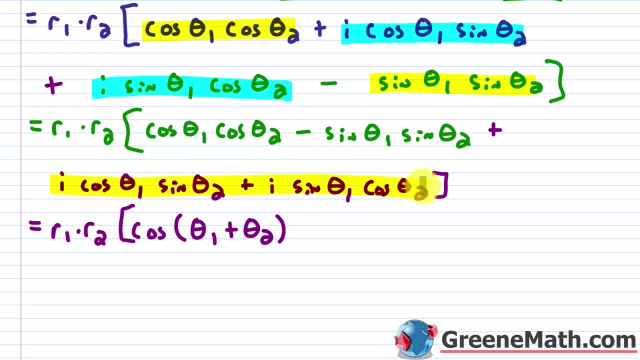 Let me highlight this: This guy plus this guy. I'm first going to factor the I out. OK, so I'm going to put plus. let me do this over here. Let me put plus and put an I there And inside what I would have is the cosine of theta sub one. 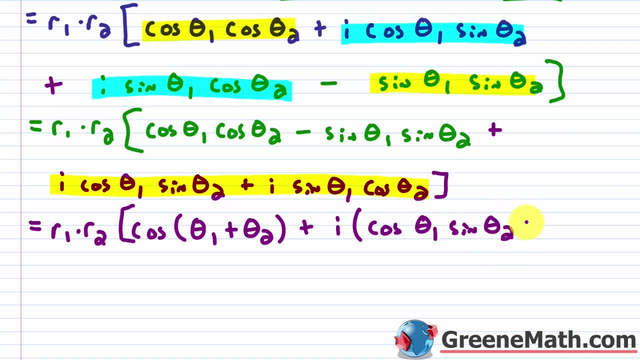 OK, times the sine of theta sub two, And then you'd have plus. you'd have your sine of theta sub one, Then times your cosine. I probably can't fit this. Let me move this down here. Let me move this down here. 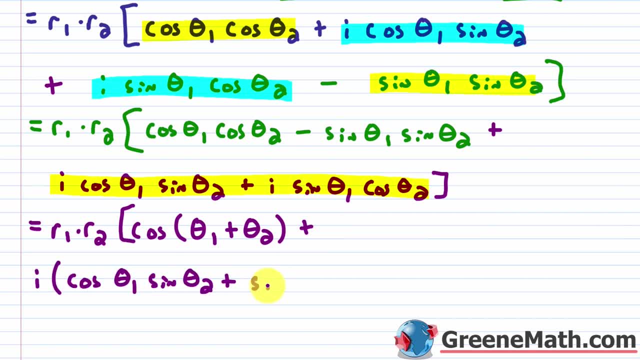 So times the cosine and make this a little bit better. So the sine of theta sub one times the cosine of theta sub two. So then let me close the bracket off here. So that's officially done, OK, and basically, you see, once I factored. 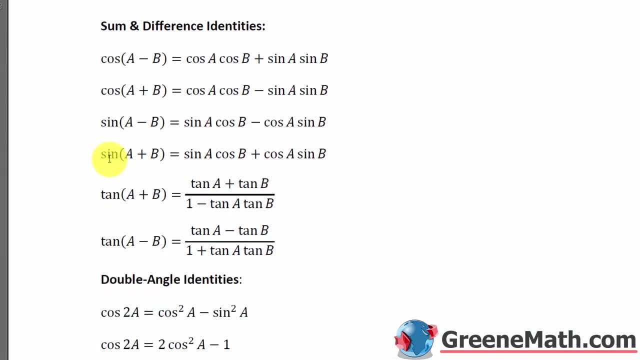 this. I out that here we can go back and we see that we have: sine of A plus B is the sine of A times the cosine of B plus the cosine of A times the sine of B. Well, we have the same thing. OK, it's the sine of theta sub one times the cosine of theta sub two plus the cosine. 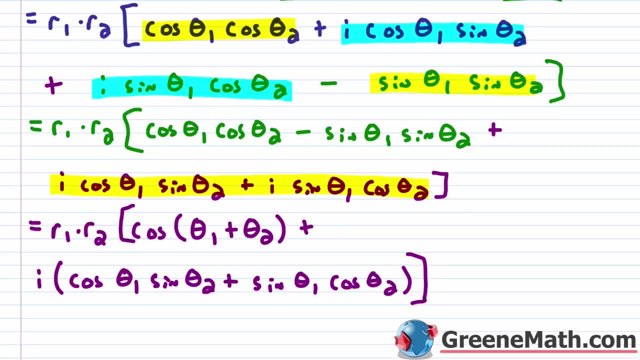 of theta sub one times the sine of theta sub two. Now, it's not in that order. OK, It's reversed here, but you could rewrite it right, because this is addition. So I could say the sine of theta sub one. 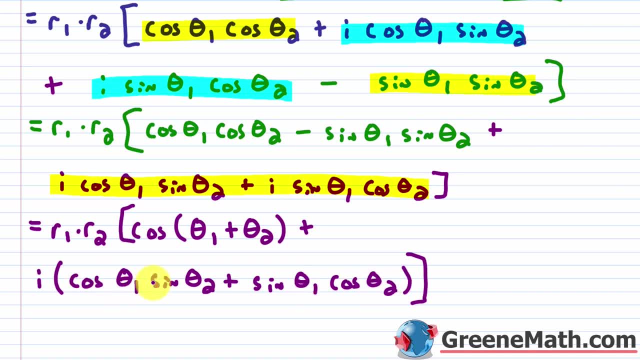 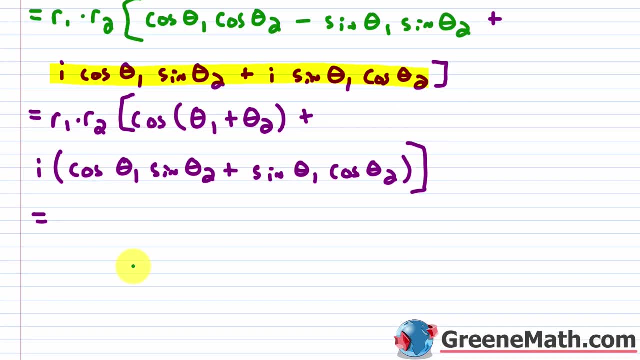 times the cosine of theta sub two, plus the cosine of theta sub one times the sine of theta sub two. OK, it wouldn't matter. So let's go and put equals. I'm going to rewrite that one as well And I'll say that I have my r sub one. 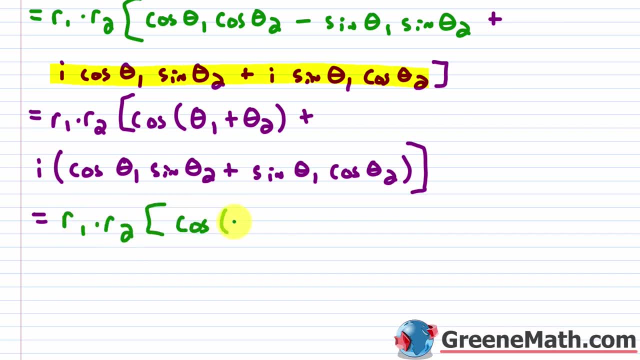 times my r sub two. inside of brackets I'll have cosine of theta sub one plus theta sub two. So then I'll say plus, I'll put my I here and I'll do my sine of. I'll say my theta sub one plus my theta sub two. 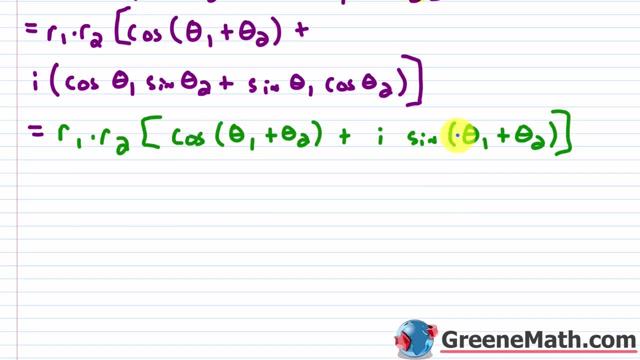 OK, let me close the brackets there. So this result here is what you're going to see when you look at your product theorem in your book. OK, so basically, you multiply the two absolute values together. That's all you need to do. 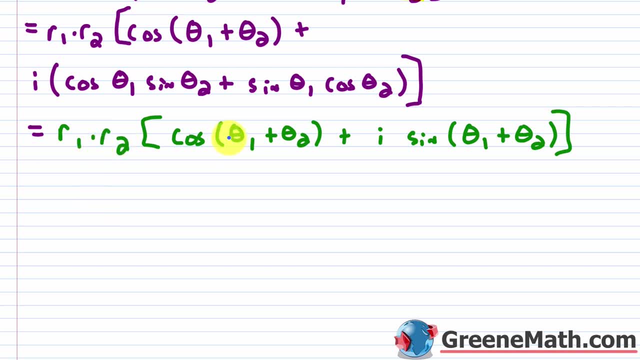 That's going to give you your r outside and then inside when you're working with this guy. you have the cosine of you're adding the two arguments together. So now it's the theta sub one plus the theta sub two plus your I times sine of. again, you're adding your two arguments together. 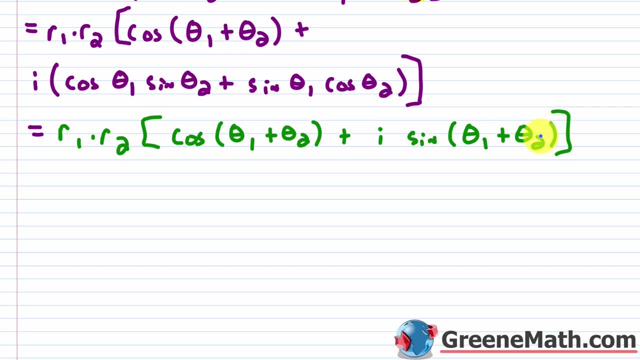 So your theta sub one plus your theta sub two. So most books will just say you're multiplying the absolute values and adding the arguments. If you want a simple way to remember that, Now another way you might see this again in compact form. 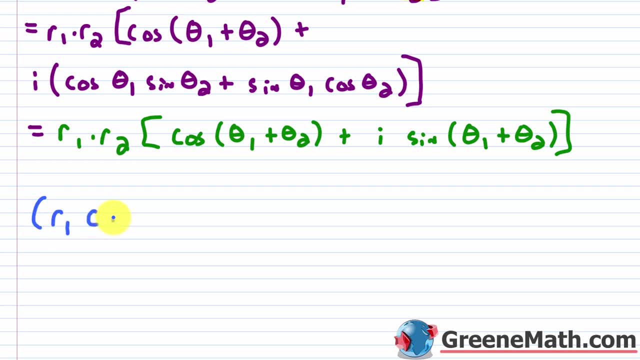 we might see this r sub one times the CIS or the CIS, right, That comes from this, the cosine, the I and the S. OK, it's an abbreviation, Let me just erase that. So basically, you have this r sub one times this CIS and I'll put theta sub one. 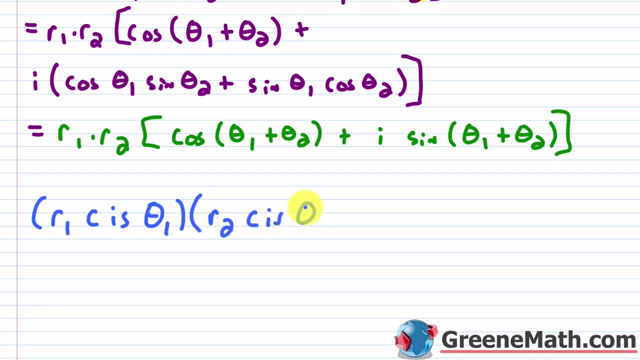 If it's multiplied by this r sub two times this CIS, and then theta sub two, this is going to be what? Again, multiply these two guys together, These two absolute values, So this is r sub one times r sub two, And then basically, you would have your CIS, and then you're adding these two. 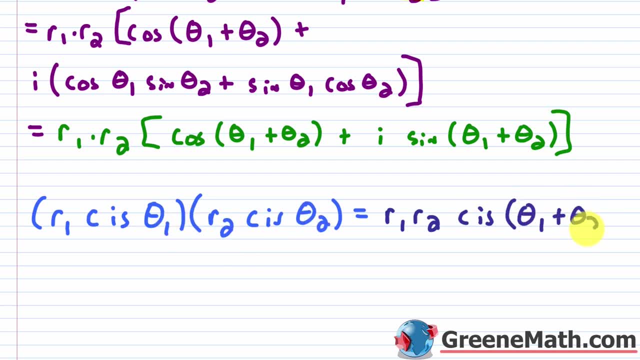 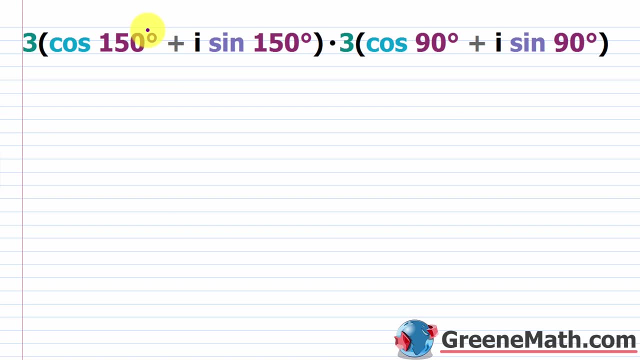 arguments together. So your theta sub one plus your theta sub two. OK, So this is the shorthand, probably a way easier way to remember. All right, So to get things started, let's go ahead and take a look at a very simple example. 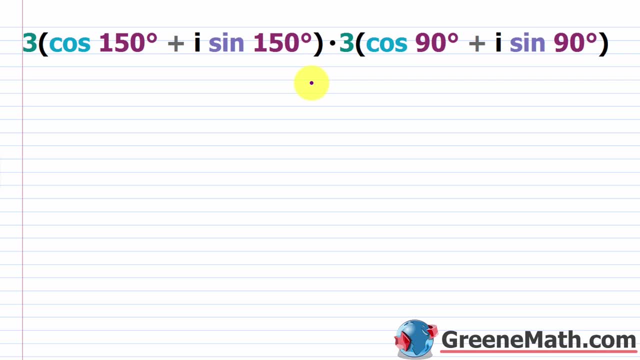 We have these two complex numbers in polar form and we just want to find the product. So we have three times this quantity. We have the cosine of 150 degrees plus I times the sine of 150 degrees. There are multiplying by. we have three. 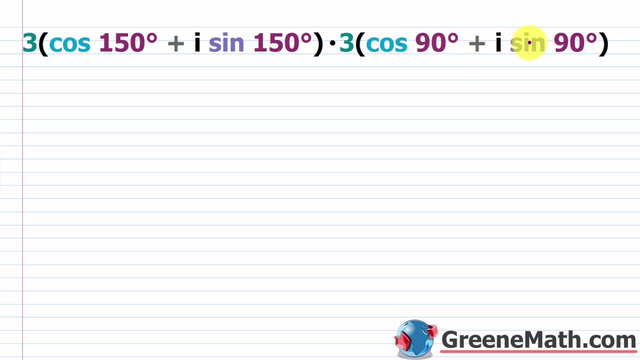 times this quantity cosine of 90 degrees, plus I times the sine of 90 degrees. So again, the very, very easy way to do this is just to multiply the absolute values together, So the absolute value of those complex numbers, So the three times the three, that's going to give me nine. 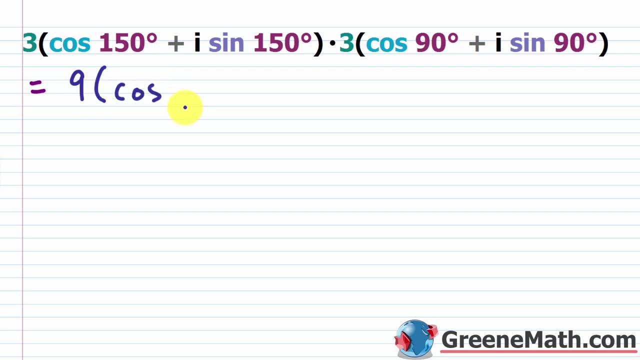 OK, And then I'm going to set this up. I'm going to go the cosine of, I'm going to add the arguments, So I'm going to add 150 degrees plus 90 degrees. That's all I want to do. So the cosine of 150 degrees plus 90 degrees. 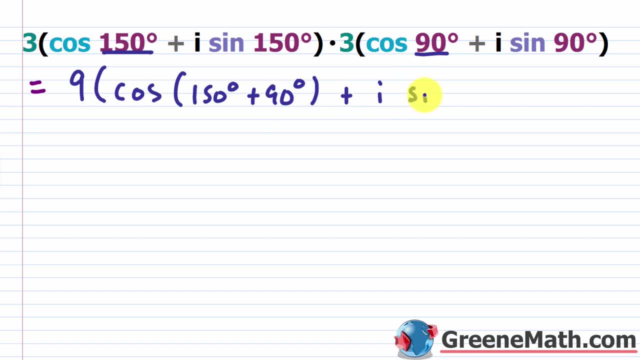 OK, And then plus my I times, I'm going to do my sine of It's the same thing, just adding the arguments. So 150 degrees plus 90 degrees, 150 degrees plus 90 degrees, OK, So basically, you're just going to simplify this. 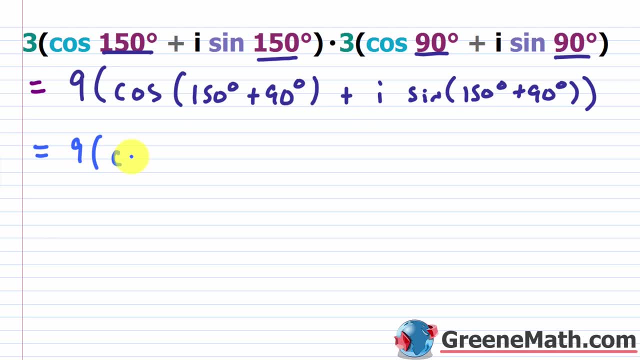 And I'm going to have nine times again this quantity. Now it's going to be the cosine of 150 degrees plus 90 degrees is 240 degrees. So I'll say this is the 240 degrees plus I times the sine of. we'll say 240 degrees. 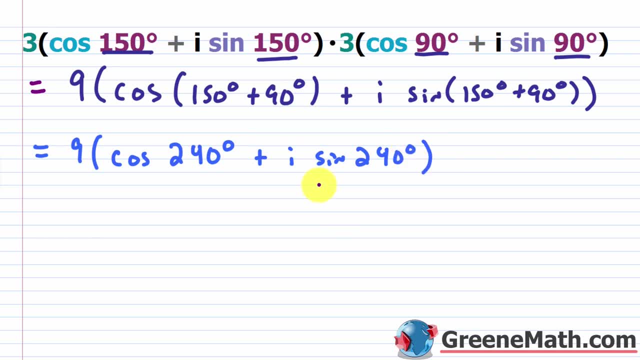 And again, you can also write this using your abbreviation, So you could say that this is the nine times the C I ask for. this is right: The C, And then the I, and then the S, and then go ahead and take that argument: the 240 degrees. 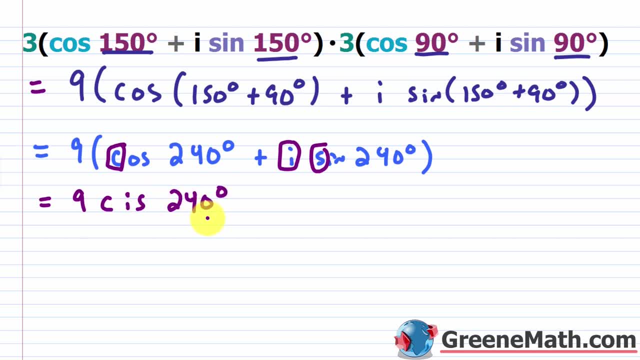 OK, that angle there. So this is another way to write it. And then, additionally, they might ask you to give it back to them in rectangular form. So let me just erase this and this and this. OK, we'll do that real quick. 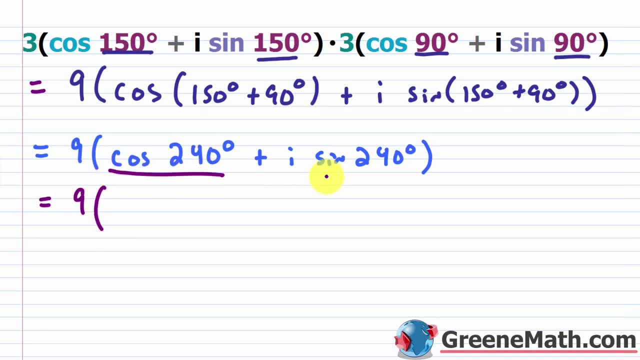 So again, for rectangular form, you need to figure out what is this and what is this, And then you're going to distribute the nine to each term inside the parentheses. So for a 240 degree angle, we have a 60 degree reference angle. 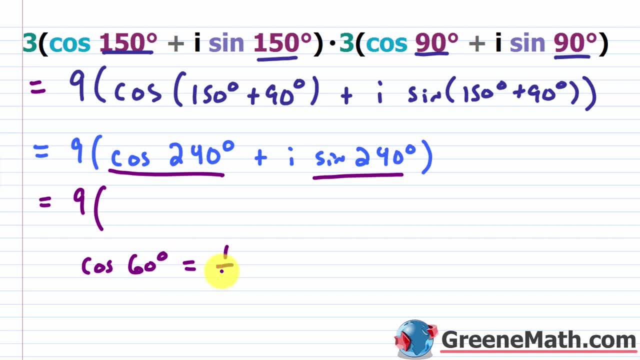 So the cosine, The sine of 60 degrees is going to be a half And the sine of 60 degrees is going to be the square root of three or two. OK, but because I'm in quadrant three, cosine and sine are both negative. 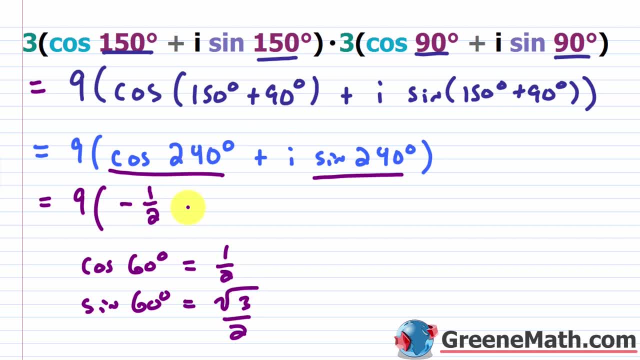 So I can say that this is negative one half, And then for this one I'll say it's negative square root of three over two. So I'll just say minus the square root of three over two And I'll just put my I behind here like this: 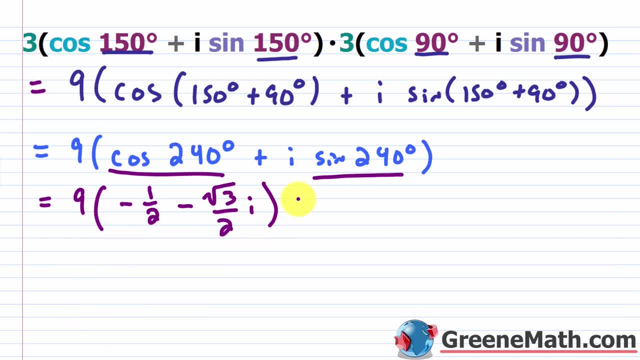 OK, so from here I'm just going to distribute the nine to each term inside the parentheses. So I would have negative nine halves like this, and then minus the nine gets distributed. So nine times square root of three over two and then times the imaginary unit. I. 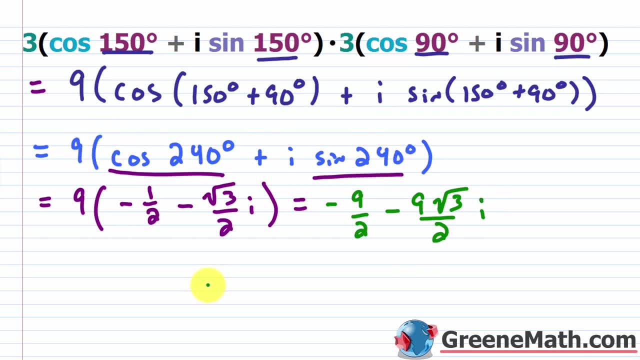 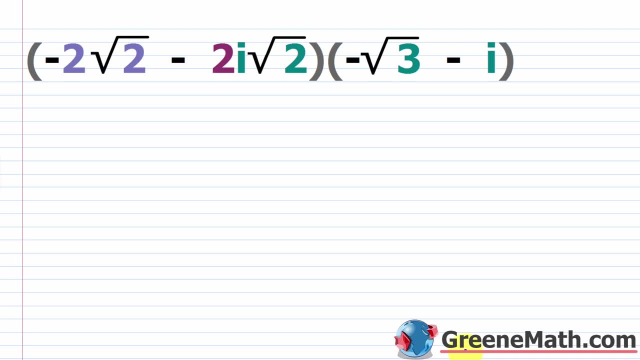 So, of course, if they ask you for polar form, it's going to be this one, OK. and then if they ask you for the rectangular form, you need to go through and figure this out and then you get this one, All right. So let's look at a slightly more tedious example. 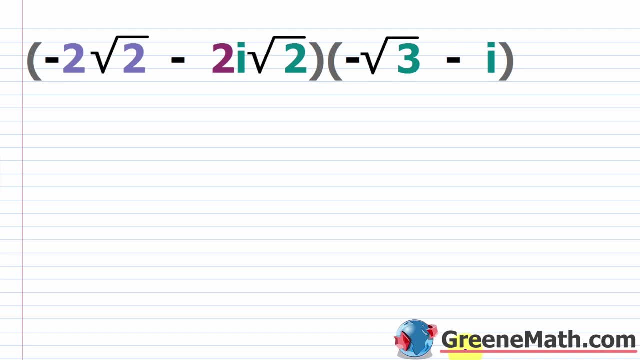 So what we're going to do here is we're going to have our complex numbers given to us in rectangular form. We're going to convert them into polar form- Just get some practice- And then we're going to use the product theorem to find the product of those two complex numbers. 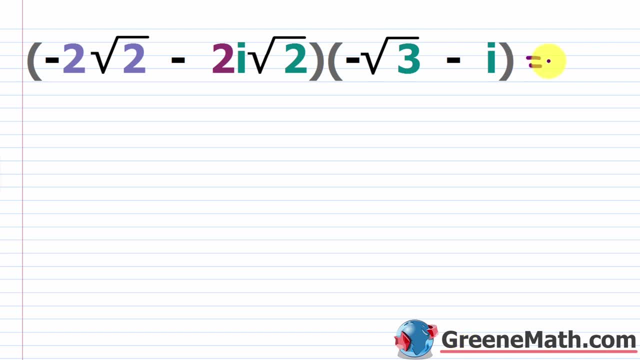 OK, so what I'm going to do here, let me put equals. I'm going to convert this one into my polar form first. So to do that, my R value would be what? Remember, that's the absolute value of the complex number. 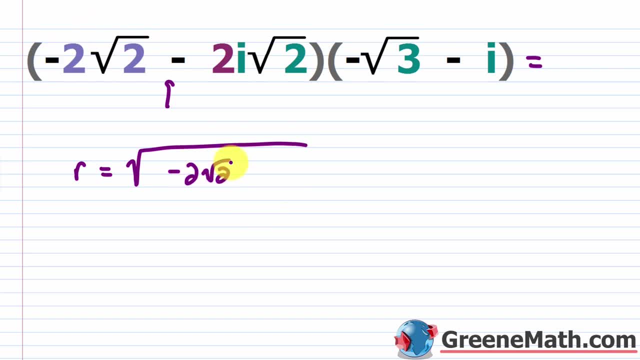 So you're going to take the real part, which is negative of two times square root of two, and you're going to square that. You're going to add that to, you're going to have your imaginary part, which is also the negative of two times square root of two. negative of two times. 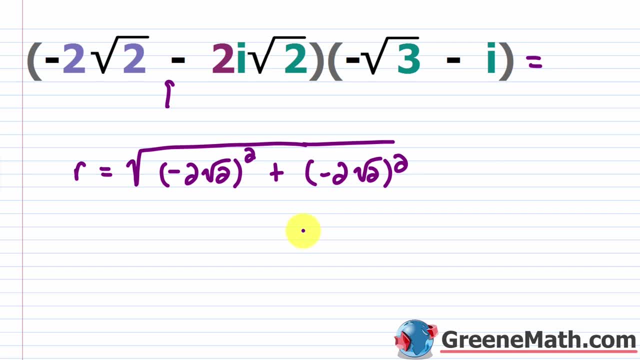 Square root of two, OK, being squared, OK. So basically, if I think about negative, two being squared, that's four. The square root of two squared is two. So in each case you have four times two, which is eight. 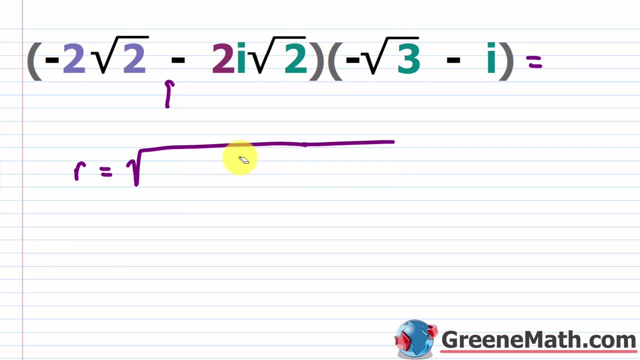 So you're going to end up with eight plus eight, which is 16.. OK, so you basically have: R is equal to the square root of 16, which is four. OK, so I can say that R equals four here. Now for the argument theta, or you could say the direction angle. 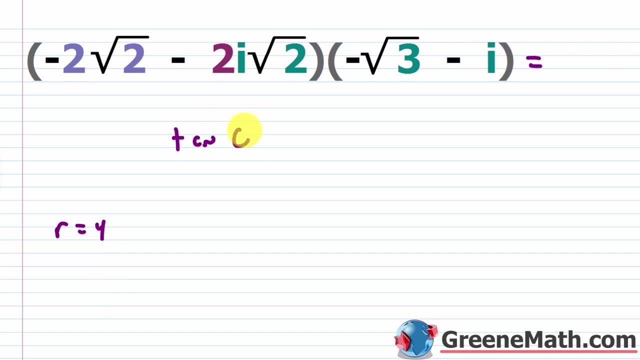 if you think about this as a vector, the tangent of this theta is the imaginary part over the real part, right, The B over the A, or you could say the Y over the X, however you think about this. So I'm going to take the negative two times. 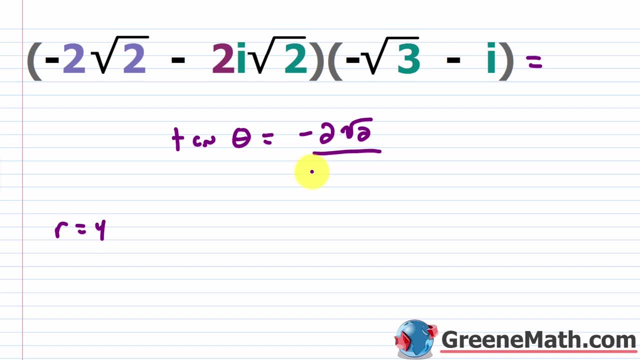 square root of two, negative two times square root of two. over negative two times square root of two. Well, this is basically going to be one, right? So the tangent of theta equals one. OK, if we use our inverse tangent function. 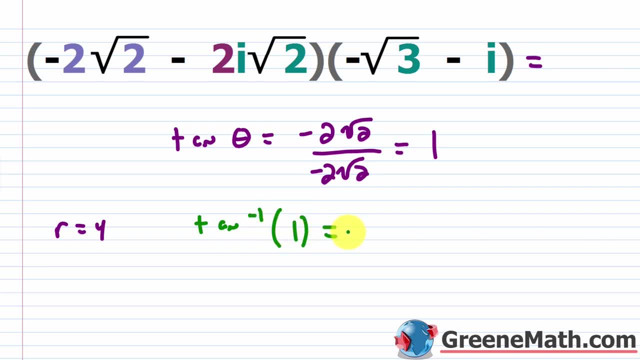 so tangent inverse of one. what is this going to give me? Well, if I'm working with degrees, I'm going to get forty five degrees. OK, but this is not our answer, Right, because, remember, we have to consider what quadrant we're in. 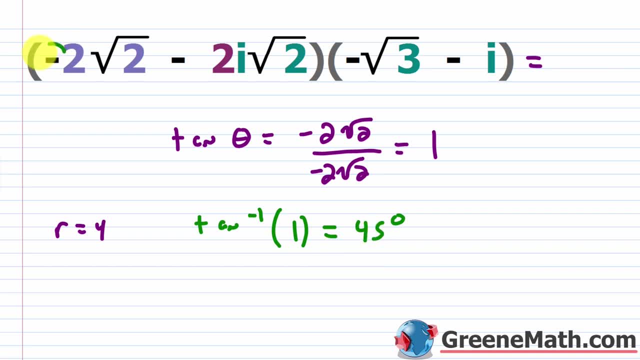 This is just going to give me the reference angle. So in this particular case, this is negative and this is negative, right? So if I was to graph this complex number on the complex plane, I would go to the left and I would go down right. 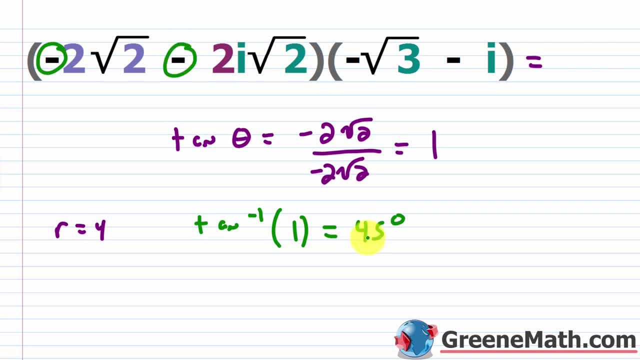 So I'm in quadrant three. So in quadrant three, if I had a reference angle of forty five degrees, I would want one hundred eighty degrees plus forty five degrees, which would be two hundred twenty five degrees. So theta here is two hundred twenty five degrees. 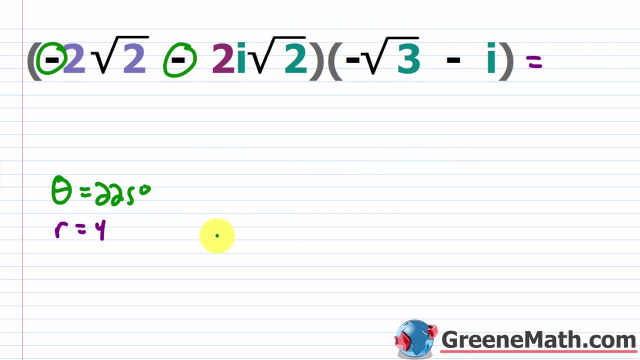 OK, so now that gives us the information to write this guy out. I can say that I R value is four. And then my argument here: theta is two hundred twenty five degrees, So I'd have cosine of two hundred twenty five degrees plus I times the sine of two hundred twenty five degrees. 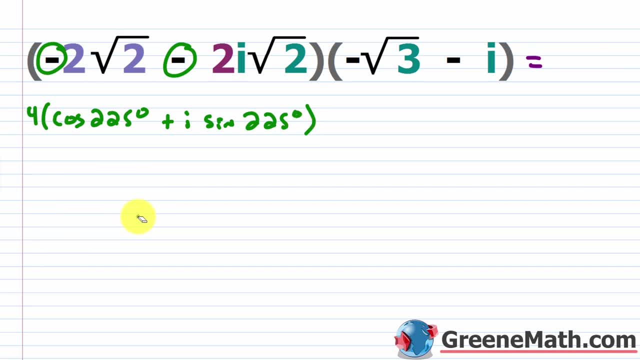 OK, so the first one's done. Now we just need to do the second one. So again, let me put times here. for this one, The R value is the square root of take the real parts of negative, of the square. three is squared, and plus take the imaginary part. 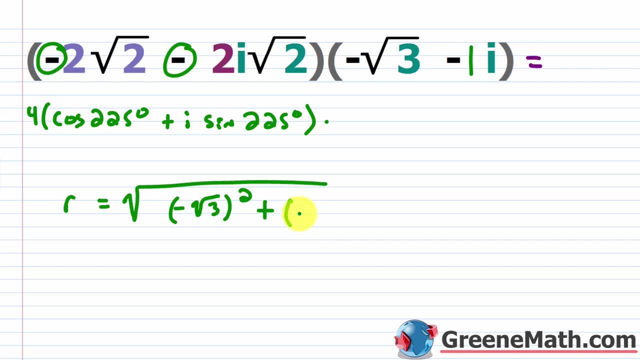 You can write a phantom One in there. This is really negative one, So I'll put negative one here and this will be squared, OK, so basically the negative of the square of three being squared is three and negative one squared is one. So you're going to have three plus one. 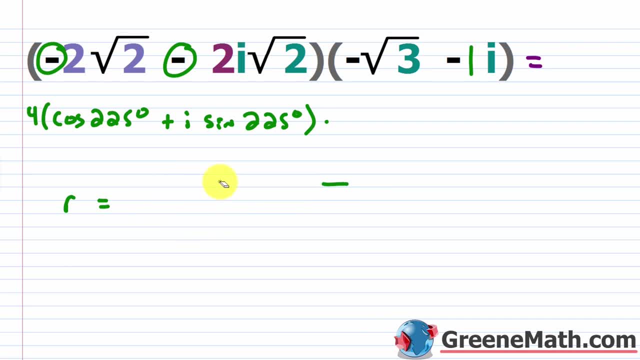 which is four. So R is the square root of four, which is two. OK, so let's put two here. And then again, for the direction angle, theta. I think about the fact that the tangent of theta is the imaginary part, which is negative, one over the real. 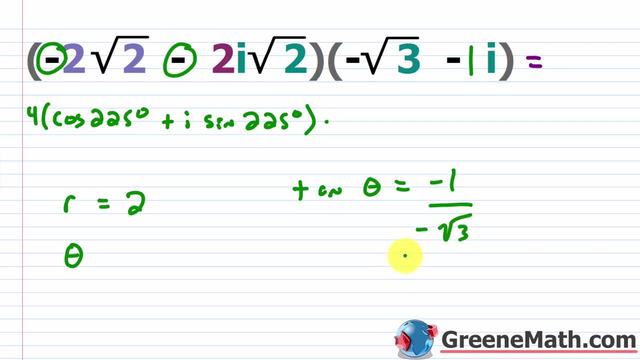 part, which is the negative of the square root of three. Now I'm going to go ahead and get rid of the negatives, So I'm just going to erase that from here And I'm going to rationalize the denominator, So square root of three over square root of three multiplied by that. 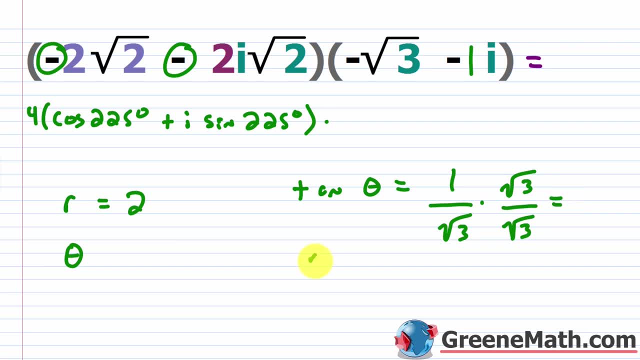 And this gives me a tangent of theta, which is going to be the square root of three over three. OK, let me erase this and actually make this a little bit more compact. So the square root, the square root of three over three. 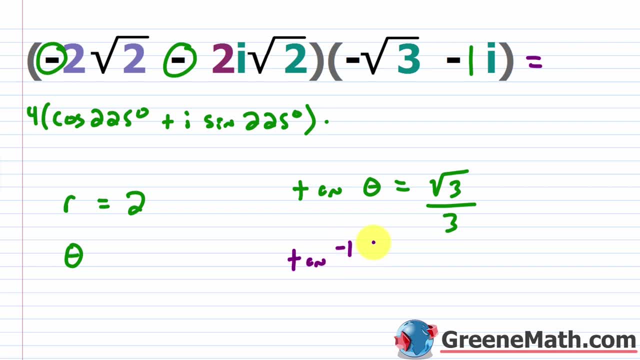 So, again, if you punch this into your calculator, if you do tangent inverse of square root of three over three, you're going to get 30 degrees. OK, but again, this is going to be a reference angle because this is negative and this is negative. 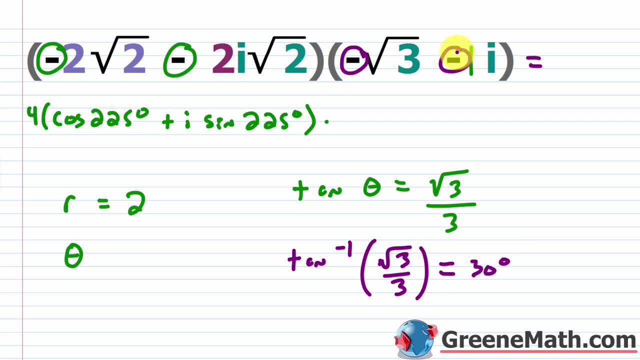 So again I'm in quadrant three, Right. If I want to plot that guy I'd have to go to the left and go down. So in quadrant three, if I have a reference angle of 30 degrees to find that I have 180 degrees plus 30 degrees, that's 210 degrees. 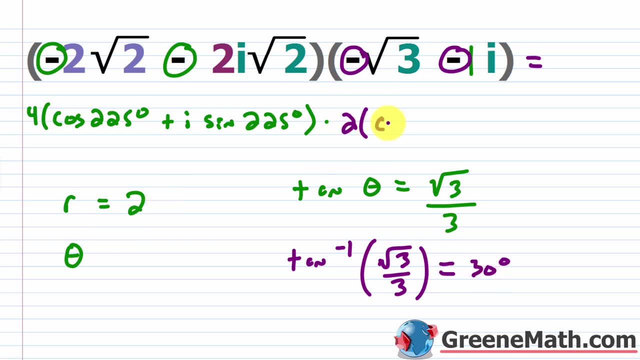 So my R value is a two. OK, put my parentheses there. I'd have cosine of, I would have. theta is 210 degrees here. OK, so 210 degrees plus I times the sine of 210 degrees, OK, And again, you can use radians if you want. 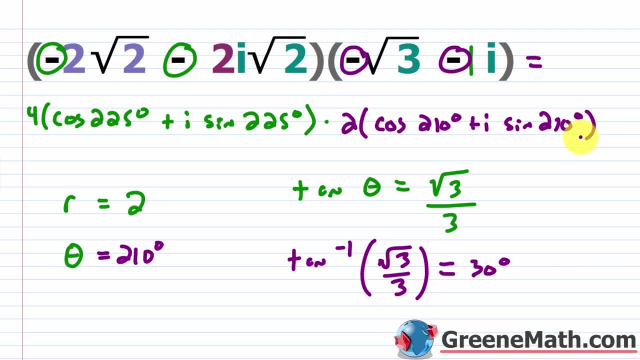 It's just a matter of what your teacher is working with. I'm just going to work with degrees here for now. OK, so now to find the product again, multiply the absolute values. So four times two is eight, And then I'm going to set this up. 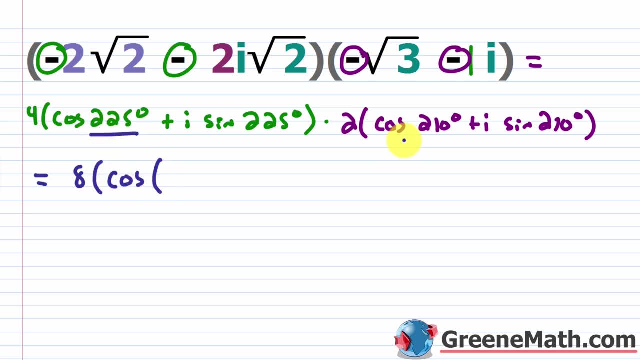 I'm going to go cosine of, I'm going to add the arguments. So 225 degrees plus 210 degrees. So 225 degrees plus 210 degrees, OK, plus I times the sine of again. I'm just going to add the arguments. 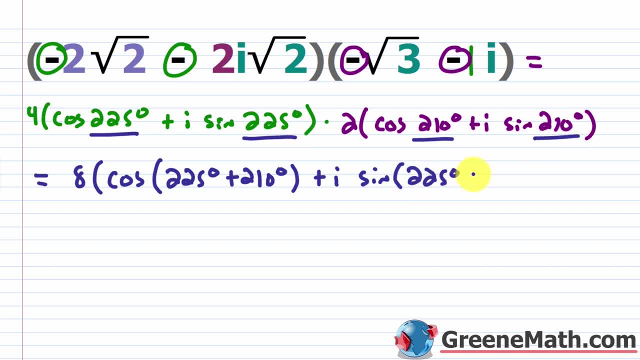 225 degrees plus 210 degrees. So 225 degrees plus 210 degrees. OK, let me close that down. So we'll say this equals eight times. OK, this quantity here is going to be the cosine of 225 degrees plus 210 degrees. 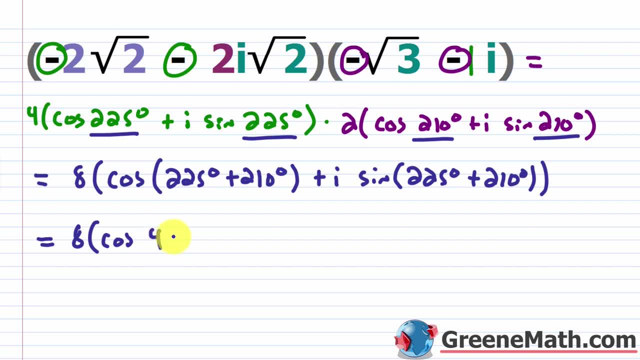 would be 435 degrees. So I'll say this is 435 degrees and then plus I times sine of again that 435 degrees. Now for some teachers this answer is fine. For others, they want you to give an angle that is between zero and 360 degrees or zero and two pi. 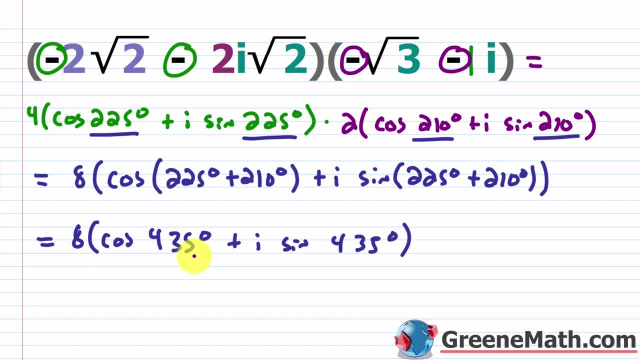 If you're working with radians, or in each case the zero is going to be included and your two pi or 360 degrees is not going to be included. OK, so basically, you would subtract this work with degrees, 360 degrees from each one of these to get your coterminal angle. 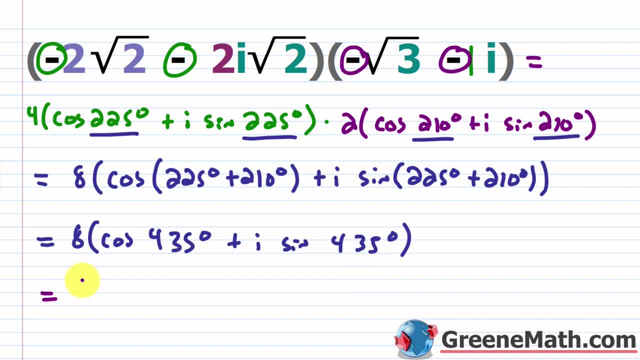 And in this case it's going to give you 75 degrees. OK, so I can say this is equal to eight times the quantity You have, the cosine of 75 degrees plus I times the sine of 75 degrees. OK, so just get with your teacher in terms of if you need to do that. 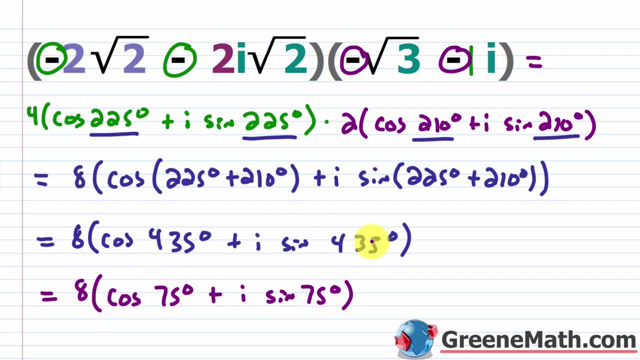 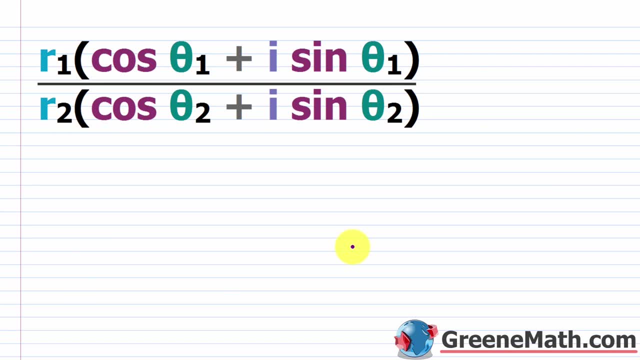 Most books will go to this. Some books will leave it like this and say it's fine, So it's really up to your teacher. All right, Now let's move on to talk about the quotient theorem. So again, I'm going to go through where this comes from. 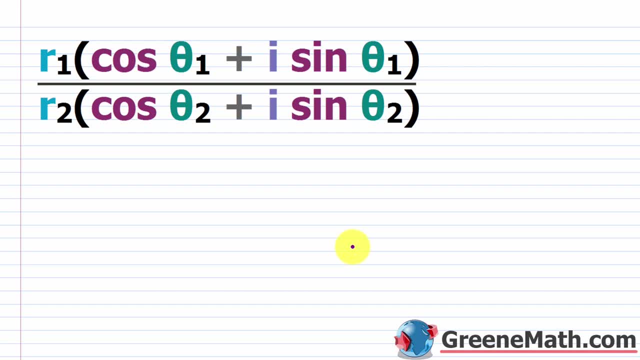 I know a lot of you find this quite boring, but it's good to be able to see where things come from. It also gives you a lot of practice with manipulating things. So let's say we have these two complex numbers in polar form and now we want 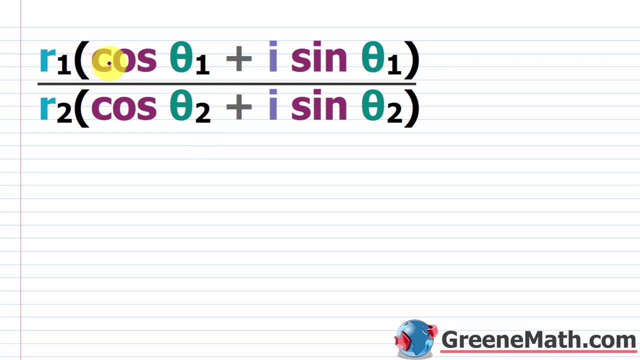 to do the division. OK, so we have this: R sub one times the quantity cosine of theta sub one, plus I times sine of theta sub one over R sub two times the quantity cosine of theta sub two plus I times sine of theta sub two. 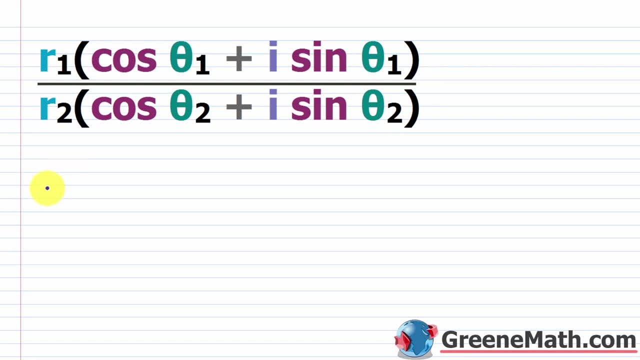 OK, let me set this up over here, because we're not going to have room to do what we need to do. So this is R sub one times the quantity, cosine of theta sub one plus I times, we have sine of theta sub one. OK, that's your numerator, your denominator here, what you're dividing by. 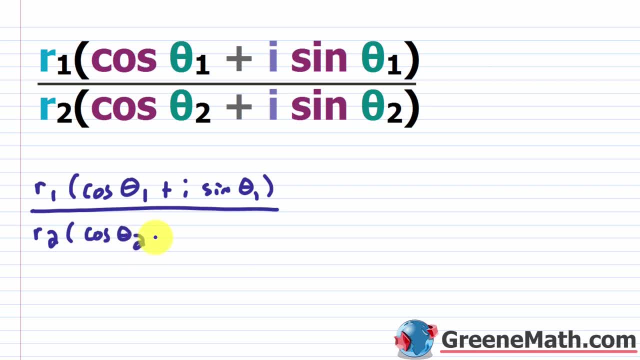 Your R sub two times the cosine of now theta sub two plus I times sine of theta sub two. OK, so the idea here is that you would multiply the numerator and denominator by the complex conjugate of the denominator. Remember if you had something like A plus. 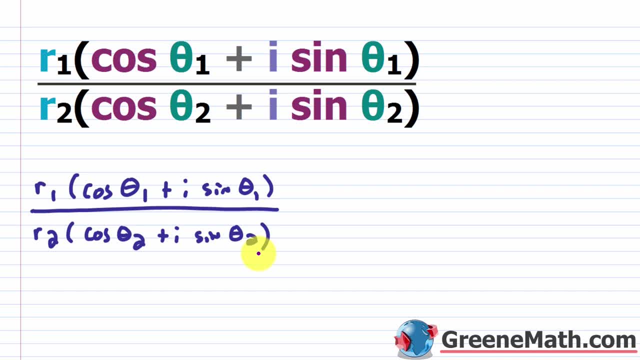 B I. the complex conjugate will be A minus B I. So here you could go through and multiply the R sub two into each term, but you end up factoring it back out. So all you really want to think about is the inside here. 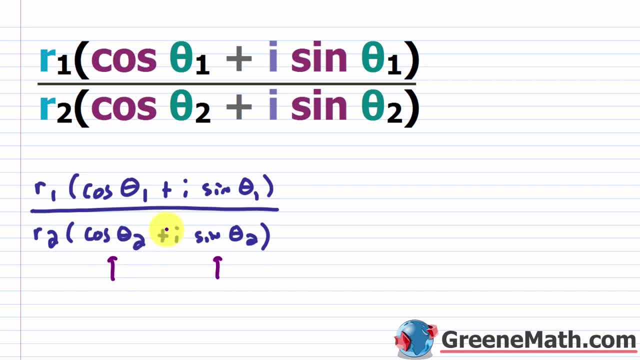 The terms are going to be the same, OK, it's just that the sine is going to be different. So what I'm going to do is I'm going to multiply by. I'm going to have this R sub two, and then times the quantity you're going to have. cosine of theta sub two. 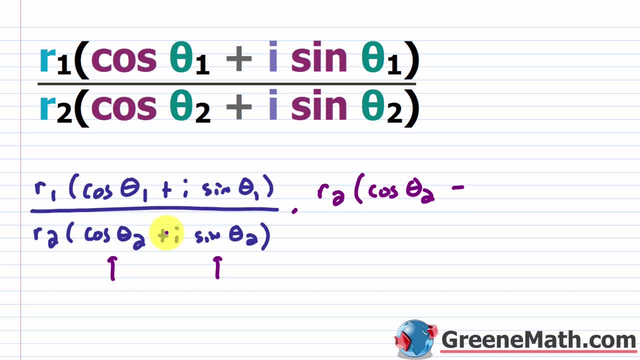 OK, so that's the same. This is going to be minus now instead of plus, And then the term is the same. So you have, I times, sine of theta sub two. Again, the R sub two here would just be factored out if it was distributed in. 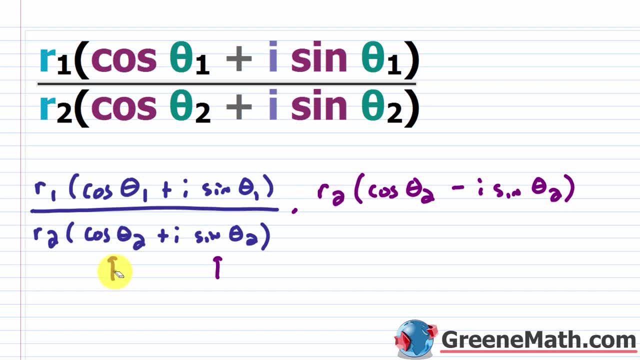 So you can think about it as just being factored out there. OK, so that's why it's out there. OK, so I'm just going to write this in the denominator here, So R sub two and then cosine of theta sub two minus I times sine of theta sub two. 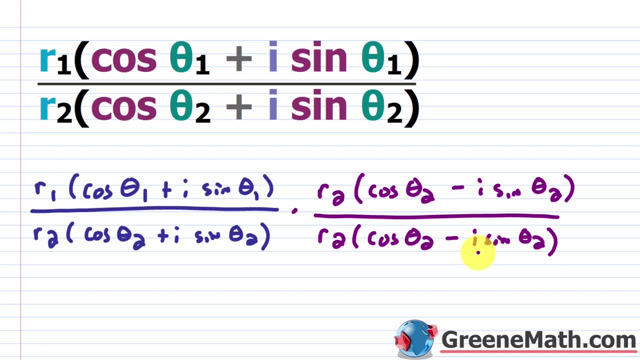 OK, like this. Now, this is quite lengthy, So I'm going to do the numerator and denominator separately. The numerator is going to be very similar to what we did earlier. It's just that we're going to have a minus involved in some different places. 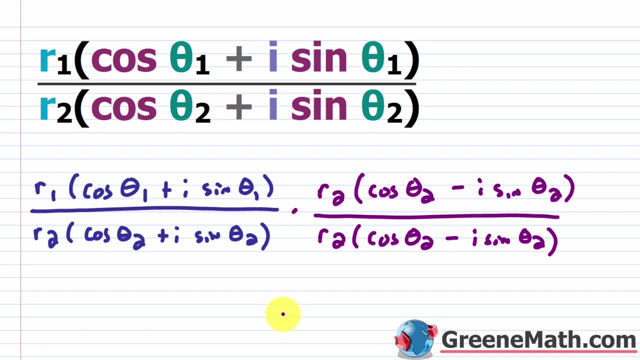 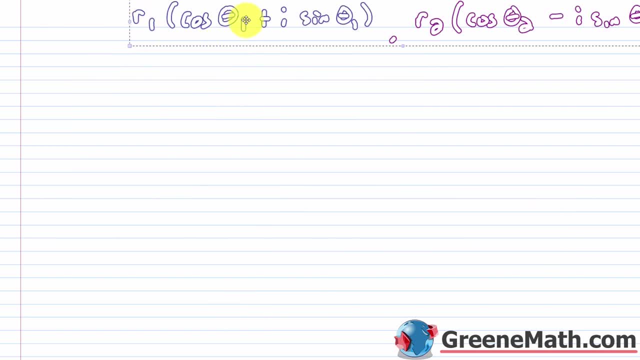 So we're going to end up using some different identities, All right, So let's go ahead and attack the numerator and denominator separately. Let me copy this, and I'm going to go to a fresh sheet here, And let me just paste this in: 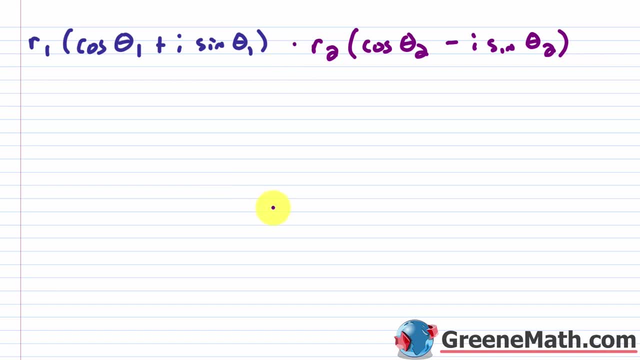 OK, And then my multiplication symbols out of whack there. So if we go through here again, we start this in a similar way to the last one, So R sub one times R sub two. OK, And then inside of here you would have: 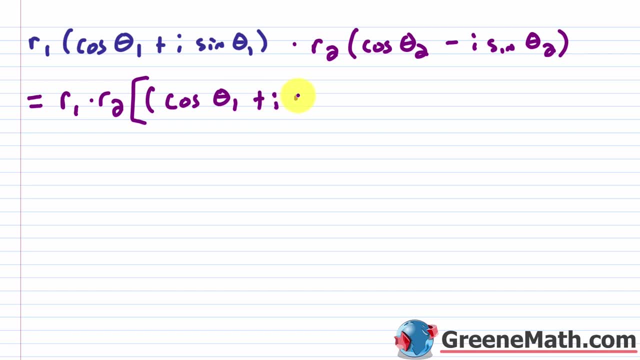 this cosine of theta sub one plus I times the sine of theta sub one, OK, And this would be cosine of theta sub two, and then minus your- I times your sine of theta sub two, OK, so again, all we're going to be doing is some simple four. 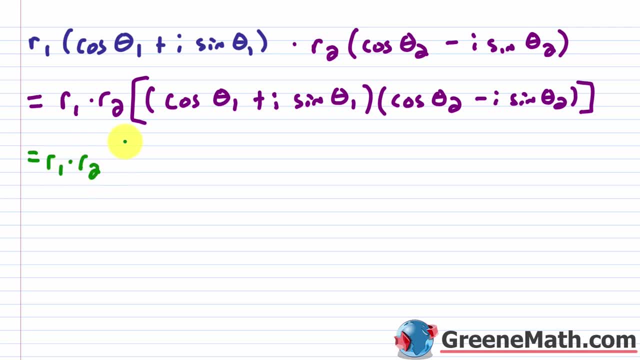 So I'm going to go equals R sub one times R sub two, like this, And I'm just going to foil things out. So first times first. So again cosine of theta sub one, and then times cosine of theta sub two. All right, So the next thing we would do is the outer. 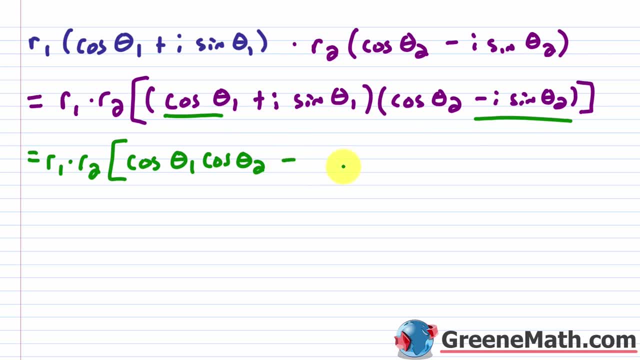 So I would do this one times this one. So I'm going to put negative, I'm going to put my eye out in front and then the cosine of theta sub one and then times the sine of theta sub two. OK, Then I'm going to go, let me erase this. 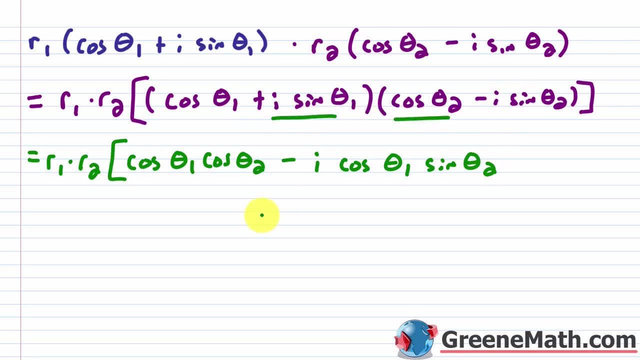 Then I'm going to go One side, So this one times this one. So I'll go plus, I'll have my eye, and then the sine of theta sub one times the cosine of theta sub two. OK, so far, so good. Now I just need my last. 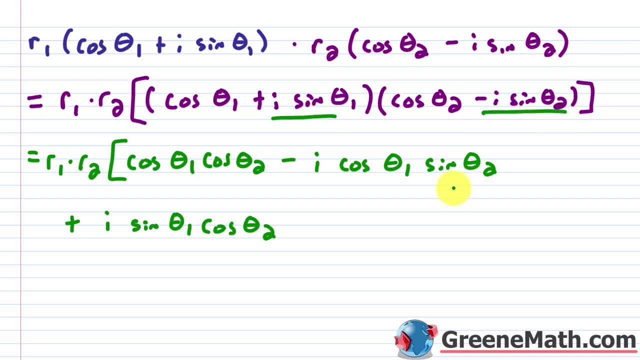 So let me go ahead and highlight This one's already done and then this one. So I know this is negative. I have I times I, which is I squared, And then I have the sine of theta sub one and then times the sine of theta sub two. 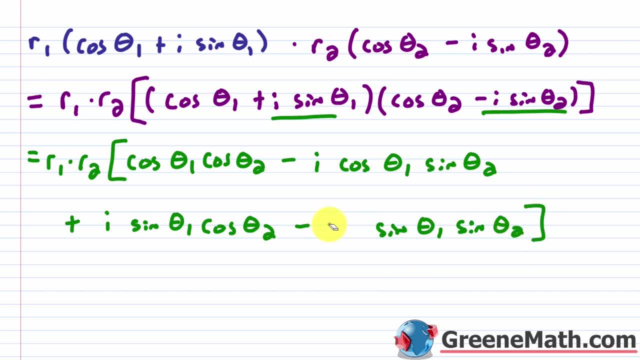 OK, let me close the bracket there, All right. So remember I squared is negative one. So this is like if we had minus, a negative one, which is basically like having plus one. OK, so you can change this, You can change this to a big fat plus. 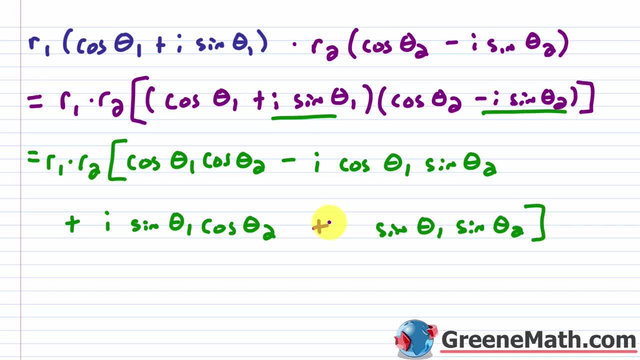 OK. so from here now, what I want to do is I want to get my terms with I together in the terms that don't have I together. So, in other words, like we did before, this will be with this OK, and let me color this differently. 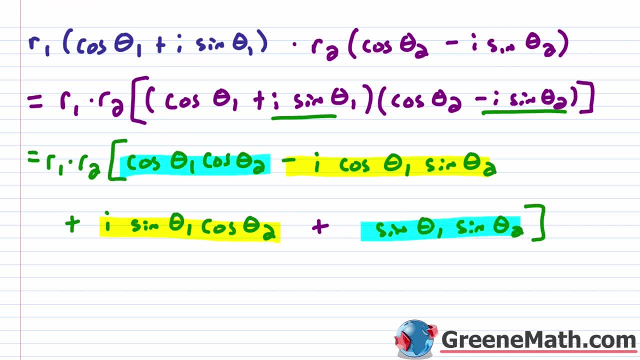 This will be with this case, So we're going to arrange it in that way. So let me go ahead and put equals here. Let me slide down just a little bit and get some room going. I'll have my R sub one times my R sub two. 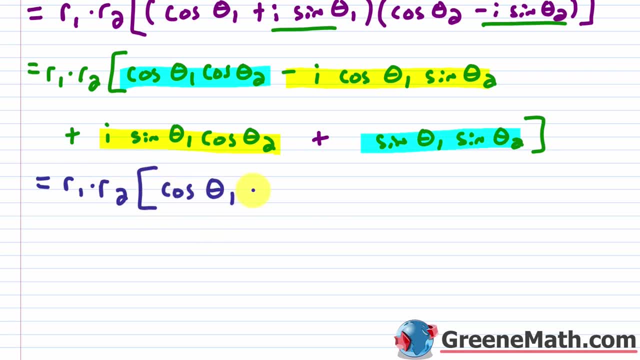 I'm going to open up the brackets. So the cosine of theta sub one times the cosine of theta sub two, OK. then I put this next: So plus the sine of theta sub one times the sine of theta sub two, OK. and then I'm going to put: you have a minus here and a plus here. 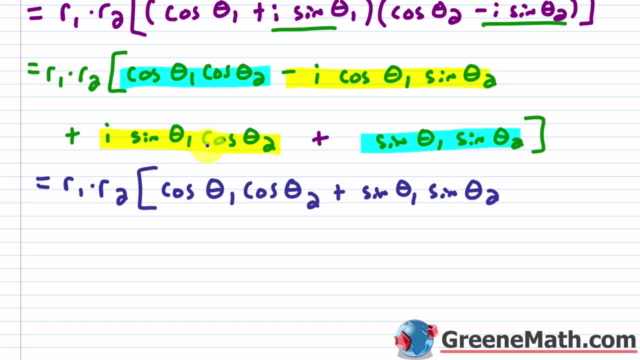 It's actually to our advantage to rearrange that. OK, you can put it like this, but in the end you can rearrange it because you're going to need an identity. So I'm just going to put this as plus. I'm going to use this one first. 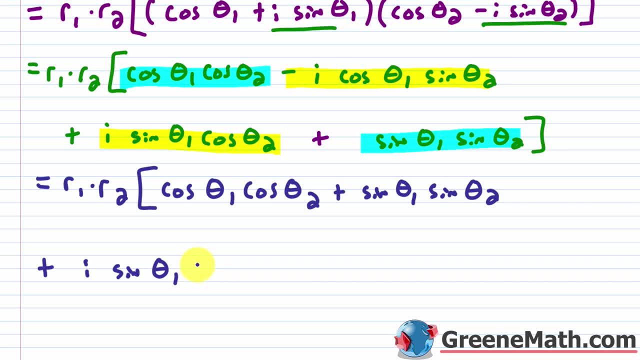 So I'm going to say I times the sine of theta sub one times the cosine of theta sub two. And then I'm going to put minus the: I times the cosine of theta sub one times the sine of theta sub two. Now you saw that last time we ended up. 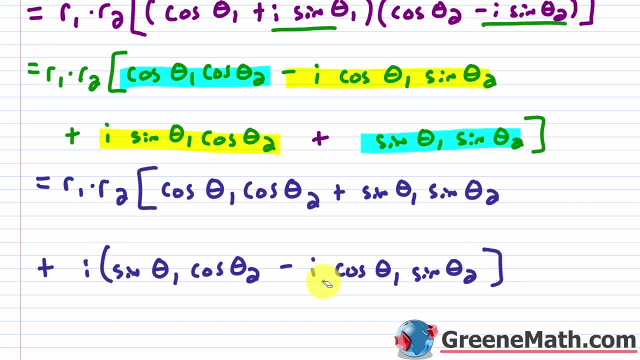 factoring the I out, So let's go ahead and do that again. So I'm going to wrap this in parentheses and I'm going to get rid of this. OK, I'm going to wrap this in parentheses as well. OK, so now what I'm going to do is I'm going to go back and I'm going to think about an identity. 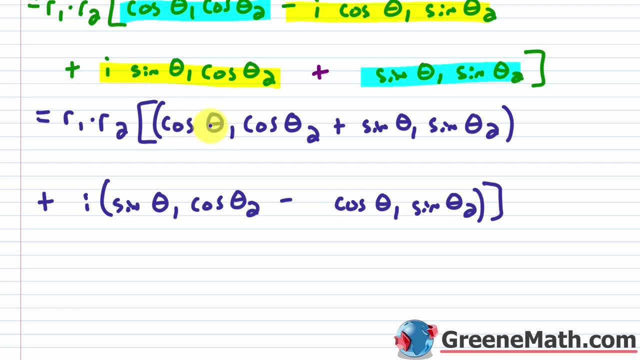 that would help me out here. So I have cosine of some angle- Let's call it theta sub one times cosine of some other angle: theta sub two. Then plus we have sine of some angle: theta sub one times sine of some angle: theta sub two. 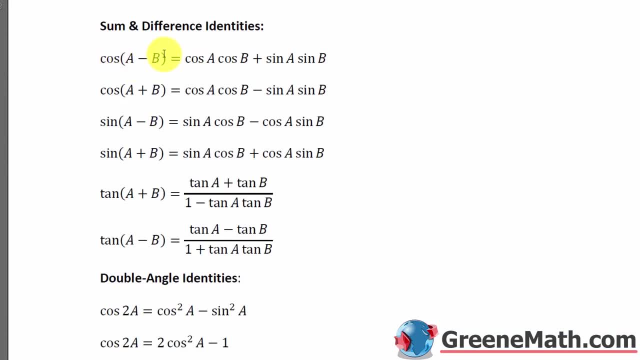 If we go back you see that cosine of A minus B follows that pattern. right Cosine of some angle A times cosine of some angle B, then plus sine of some angle A times sine of some angle B. So I can use that to rewrite this. 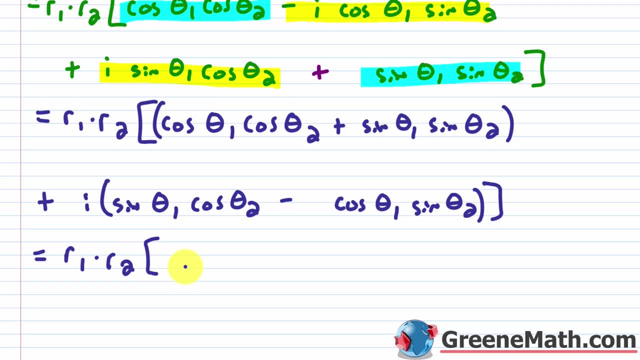 I'm going to go R sub one times R sub two And then inside of brackets here I'll have cosine of. I'll go ahead and say now this is the theta sub one minus the theta sub two. OK, so that part is done. 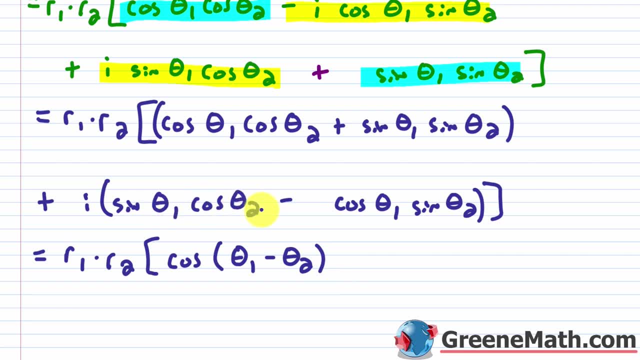 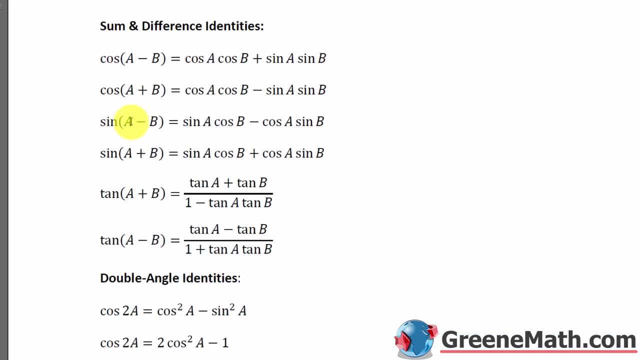 Now, when we look at this, one sine of theta sub one times cosine of theta sub two, minus cosine of theta sub one times sine of theta sub two- If we go back- that's this guy right here, right- Sine of A minus B. 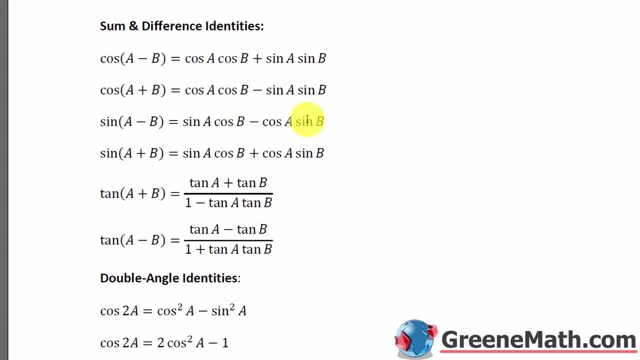 This is sine of A times cosine of B, minus cosine of A times sine of B. That's why I had to rearrange things, because it would have been this way: The minus first and the plus. You can always rearrange it, but it might not be obvious. 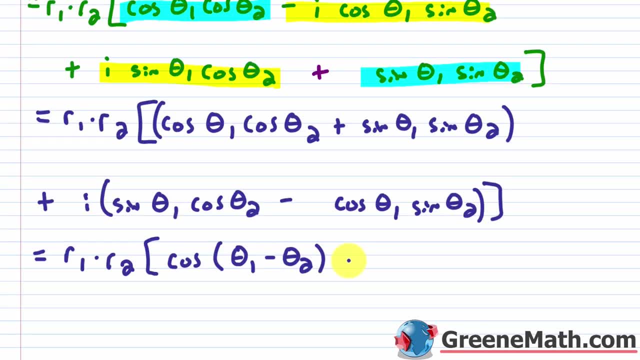 So that's why I did So. let's go back and now let's write this as plus, Don't forget the I, and then times your sine of this is going to be your theta sub one minus your theta sub two. OK, so go ahead and close this down. 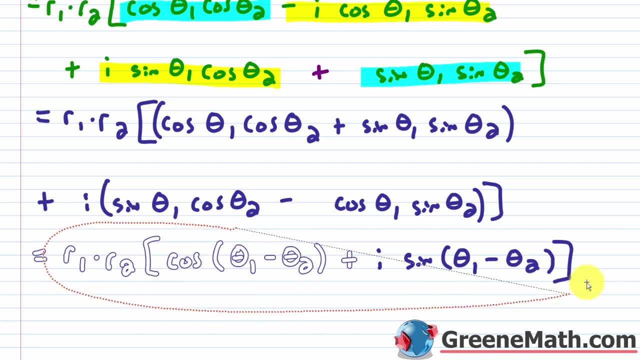 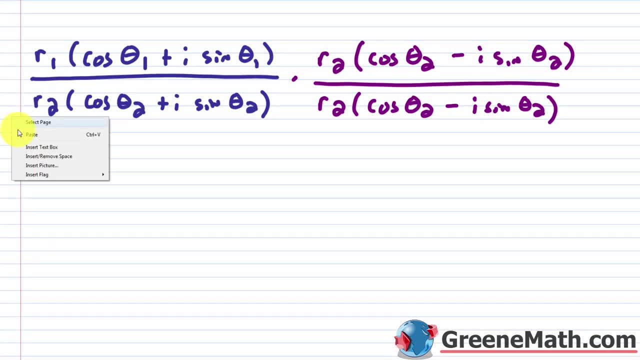 So this is your numerator. If you want to copy this, let me go ahead and copy this, And I'm back on this screen now, So let me come down a little bit. I'm going to put equals here and let me go ahead and paste that in. 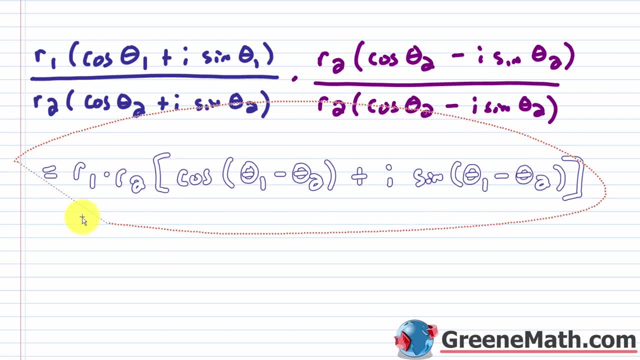 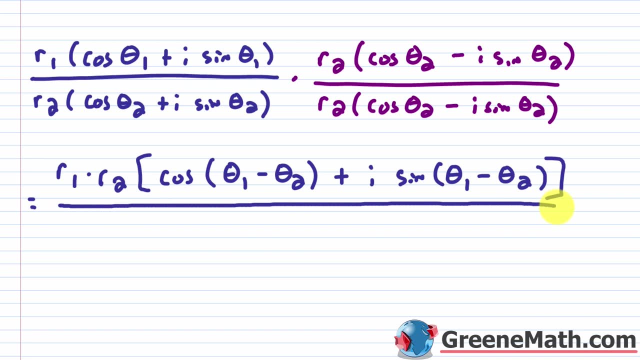 And I already had an equal, so I'm doing it twice. Let me go ahead And move this over just a little bit. So I'm going to say this equals this and actually may put this a little bit further down, and then I'm going to put this over. 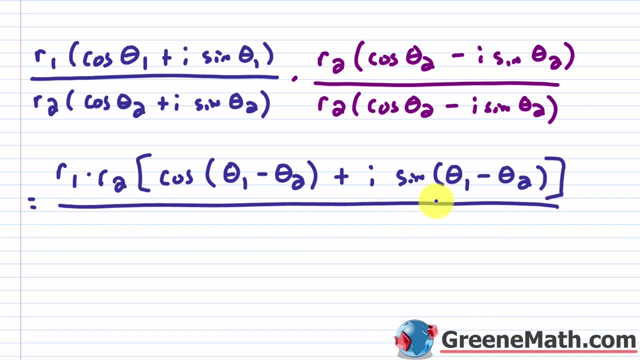 We now need to work on the denominator. OK, so let me go ahead- And actually I should probably have equals here to make this complete- And let me grab this denominator now. Let me copy it, Let's go to another sheet and let me paste this in now. 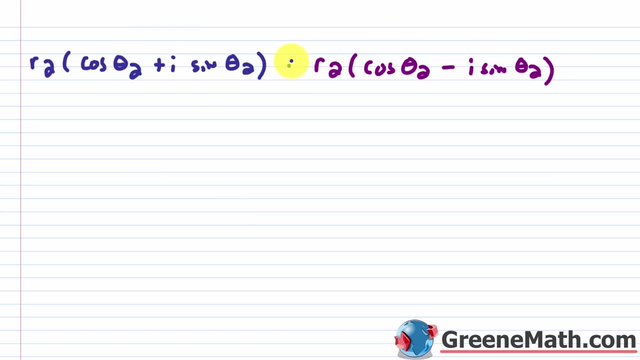 OK, and we don't need this and I need a times here. OK, so for this guy, what you need to realize is that you could first multiply your R sub two times your R sub two, So that's going to give me R sub two. 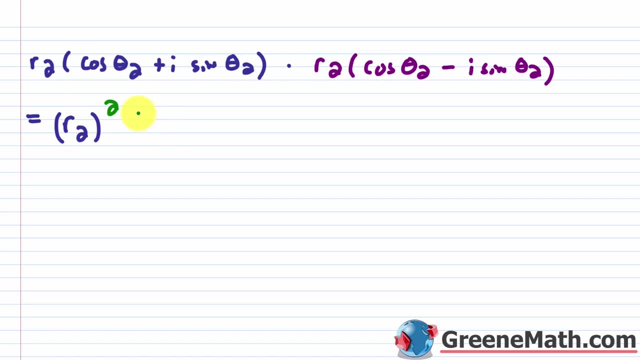 I'm going to wrap this in parentheses for clarity. So this is going to be squared, And then we're going to have the cosine of theta sub two plus I times the sine of theta sub two. OK, then times the cosine of theta sub two. 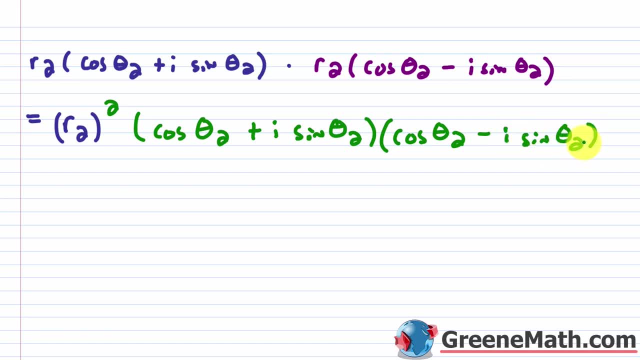 Now minus the I times the sine of theta sub two. So notice that you have these complex conjugates here, OK, because you have the same term here, OK. and then you have the same term here and here, And this looks really weird. 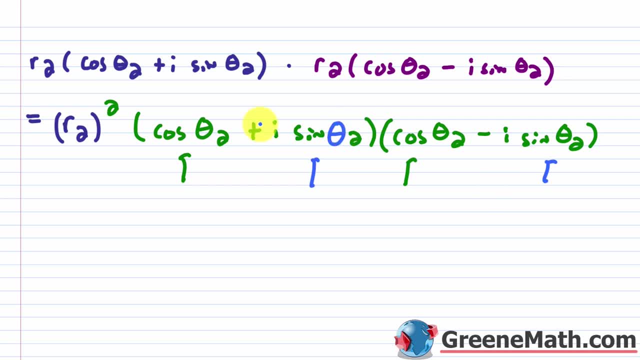 It looks like a face, So let me make that like that, And then, basically, your signs are different. OK, so what I would do here is just use my formula. So I would go ahead and say: this is R sub two being squared times. 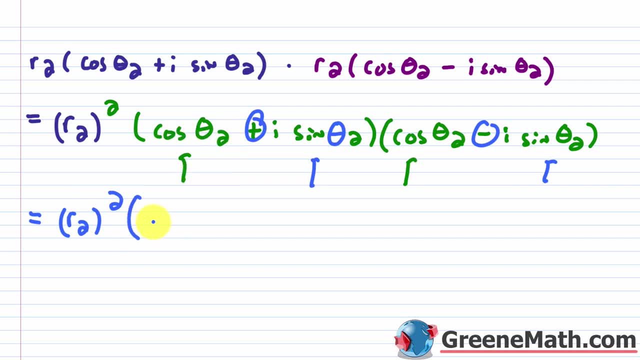 Essentially I would do the first guy squared. So let me put this inside of parentheses- I would say cosine squared, theta sub two OK, and then minus your second guy being squared. So if I squared I I would have I squared. 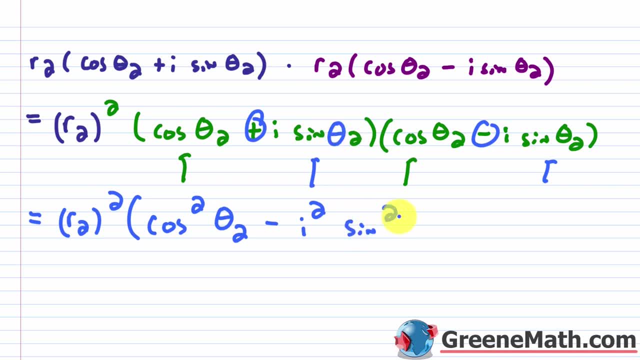 If I squared sine of theta sub two, I would have sine squared theta sub two. OK, like this. Now what are we going to do from here? Just think about this. for a second Minus I squared- Remember this is negative one. 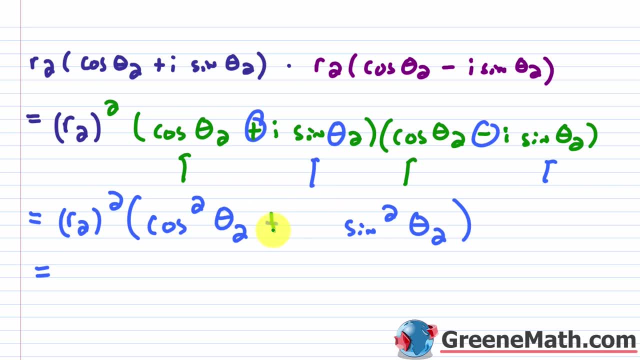 So this is basically like minus, a negative one which is basically plus. Now- hopefully you see this right away- You have cosine squared theta sub two plus sine squared theta sub two. What is that? That's one. If you go back, you see for the pi. 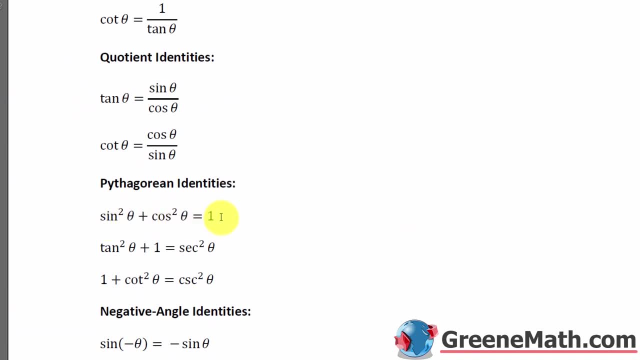 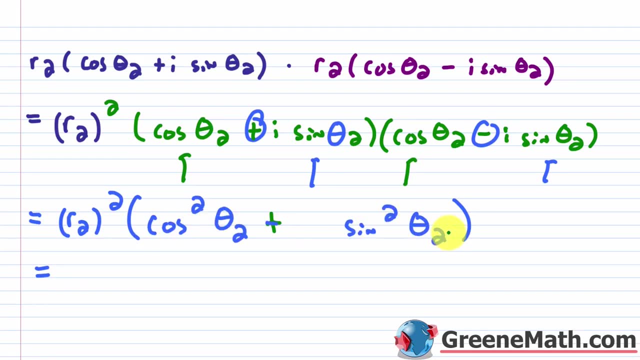 gorean identities: sine squared theta plus cosine squared theta equals one, Right? So here we have cosine squared of theta sub two, whatever that angle is, plus sine squared of theta, sub two, Same angle, whatever it is OK, And so this is going to be one. 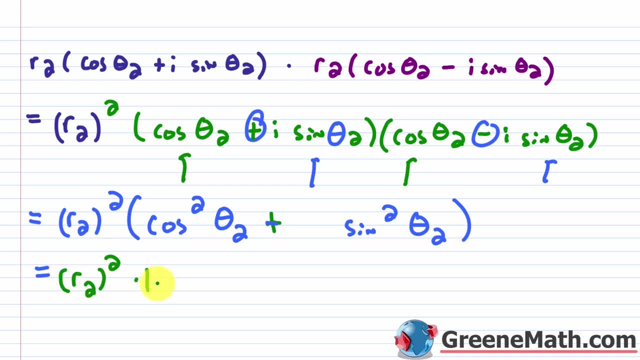 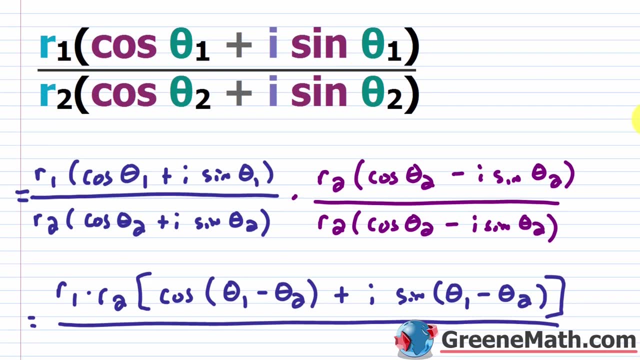 So I can say this is R sub two being squared times one, which is equals R sub two being squared. OK, so if I go back up, this is going to be my denominator, So let me bring this down here and I'm just going to put this over: R sub two. 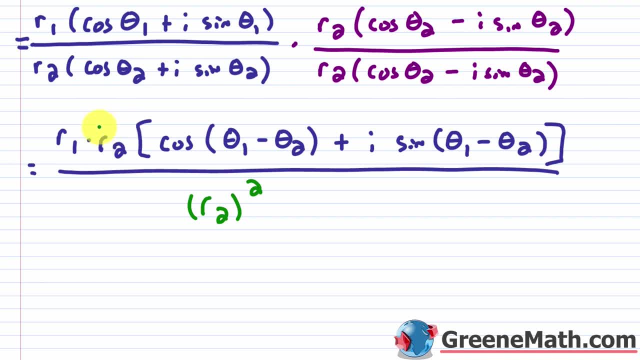 And this is squared OK. So remember, this is multiplication here. This is being multiplied. You can wrap this in parentheses to make that clear. This is being multiplied by this, So I can cancel a common factor of this guy with this guy. 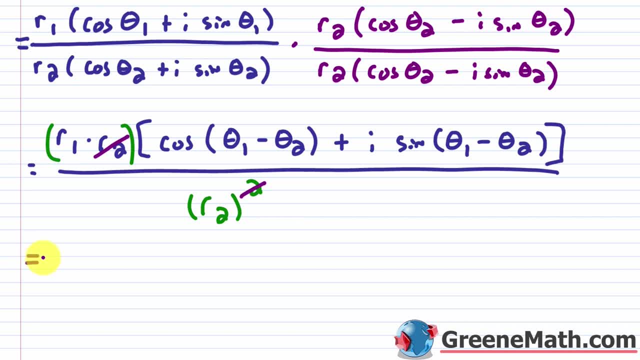 So essentially what I have here, OK, is going to be what you're going to see for your quotient theorem in your book: your R sub one over your R sub two. OK, so you're dividing the absolute values and then times this quantity here. 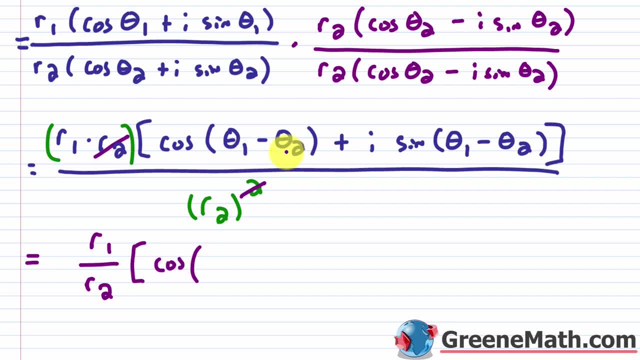 You have your cosine of you're subtracting the arguments. OK, so I'm doing my theta. So one minus my theta sub two. OK, then plus I times the sine of: again I'm subtracting the arguments. So theta sub one minus my theta sub two. 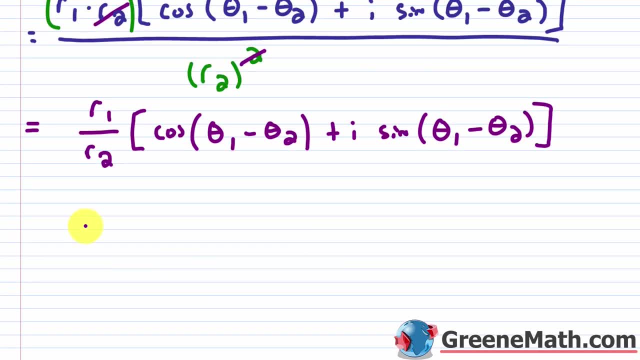 And again, if you want to write this in a more compact form, well, if you had R sub one times your size of theta sub one, divided by R sub two times your size of theta sub two, OK, what this would be equal to is your R sub one over your R sub two times. 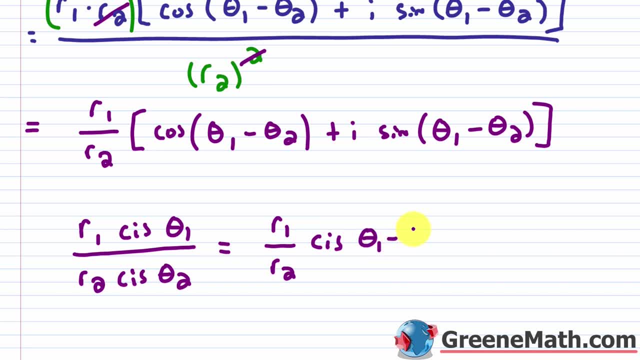 your size of your theta sub one minus your theta sub two. OK, so we can wrap that in parentheses And that's basically the shorthand. I think this is the easiest way to remember things, And let's just go ahead and look at an example. 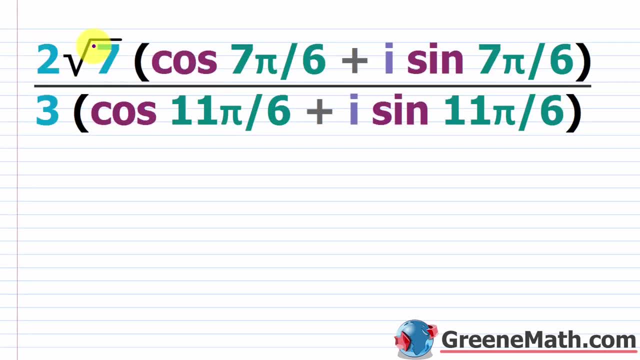 All right. So what we'll do here, we'll have this two times square to seven times the quantity of the cosine of seven pi over six, plus I times the sine of seven pi over six and this will be over. you have your three times the quantity. 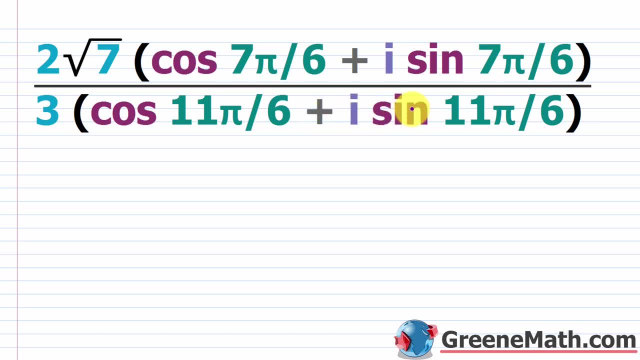 of your cosine of eleven pi over six, plus I times sine of eleven pi over six. So of course these two complex numbers are in polar form, so we can immediately use this quotient theorem. OK, but to get a little bit of extra practice, let's write our answer in polar. 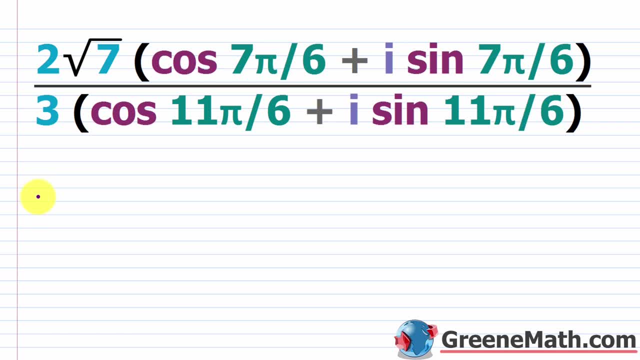 form first, and let's also go into rectangular form. OK, so let's go and say this is equal to: I'm going to divide the absolute values. So I'm going to say two times square to seven or three. OK, this is going to be times the quantity. 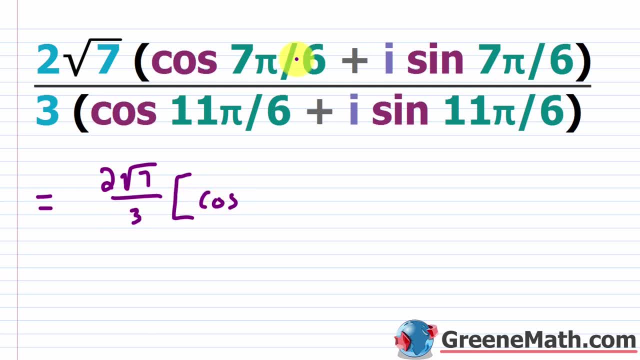 What you're going to do here is you're going to have your cosine of. you're going to do is you're going to divide over seven pi over six minus eleven pi over six, and I'll take care of this in a moment. I'll just leave it like this for now. 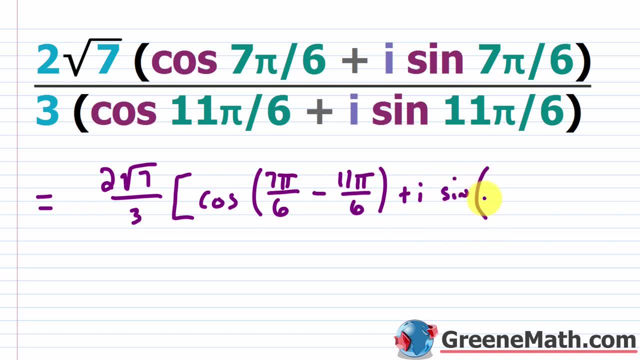 And then plus I times your sine of, again you're doing the same thing. So seven pi over six minus eleven pi over six. OK, so just like that, All right. So let me close this down. So that's proper. Let's put equals here. Let me scroll down and get a little bit of room going. 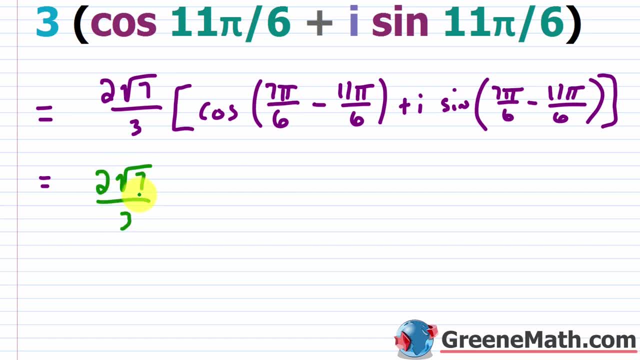 So let's go ahead and say we have two times square to seven over three. okay, let me make that 3 a little bit better. and then inside of here I'll have the cosine of: if I do 7 pi minus 11 pi, that would be negative 4 pi. right, you already have a common denominator. so 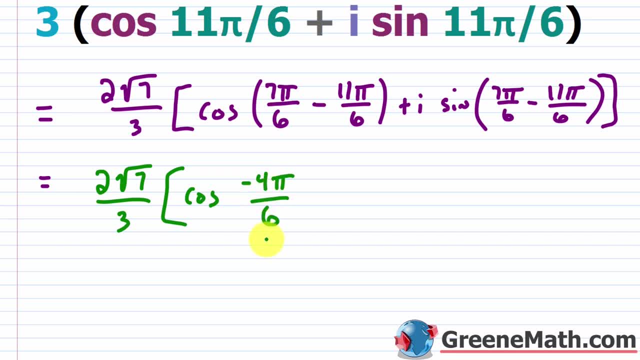 let's say this is negative: 4 pi over 6, and of course you can reduce the fraction. each is divisible by 2, so this would be 2 and this would be 3. so this is negative: 2 pi over 3. okay, then I'll do. 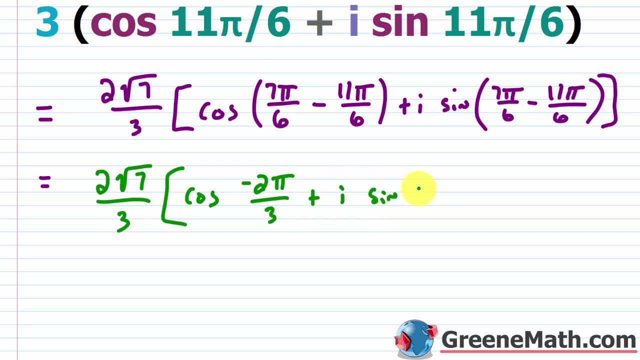 plus i times sine of the same thing. right, it'll be your negative, your negative. 2 pi over 3. let me go ahead and write this down here like this, and let me go ahead and close the bracket there. okay, so again, some teachers will accept this. some of them want you to find the coterminal angle. 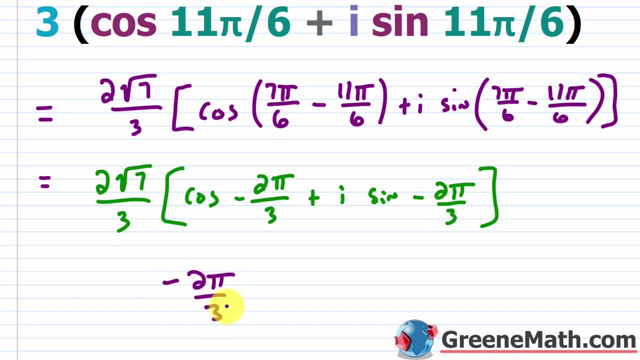 so what I would do here is I could say negative: 2 pi over 3 plus 2 pi, right. or if I want a common denominator, this would be: multiply this by 3 over 3, so this would be 6 pi over 3. okay, so 6. 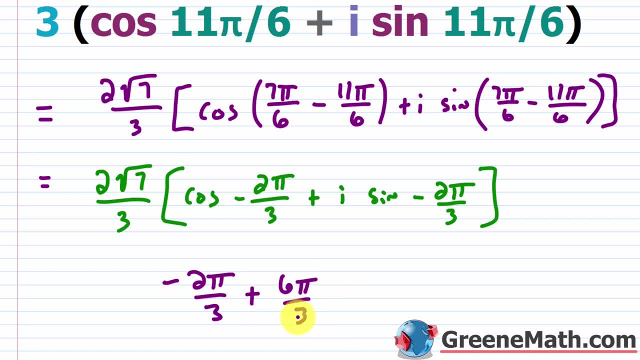 pi over 3.. So your coterminal angle here would be 4 pi over 3.. So you could really write this and you could say that this is 2 times square root of 7 over 3, and then inside the brackets I'll say: this is the cosine of 4 pi over 3, okay. plus i times the sine of 4 pi over 3, okay, So for: 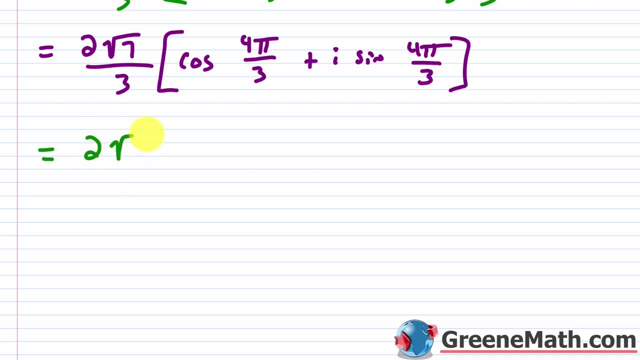 your rectangular form. what we'll do is we'll have 2 times square root of 7 over 3.. We need to think about the cosine, the cosine- let me make a border here- the cosine of 4 pi over 3. okay, So this is: 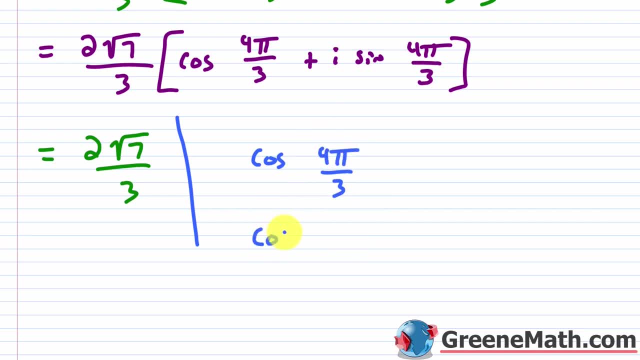 going to be 240 degrees if you convert it into degrees. so cosine of 240 degrees, that's easier for you. Again, it's going to have a 60 degree reference angle, or pi over 3 in terms of radians. So if you think about cosine of 60 degrees, again it's a half right and this angle here, 240 degrees. 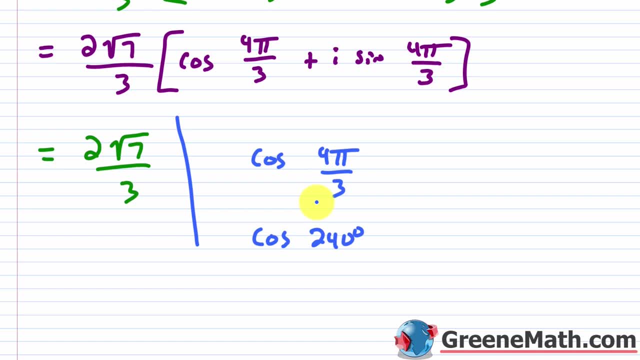 or 4 pi over 3. that's going to be in quadrant 3.. So we know cosine is negative there. so this would first be the negative of a half. So let me put some parentheses here and say this is negative one half. Let me put plus my i so I don't forget it If I think about the sine of 4 pi over 3 again, 60. 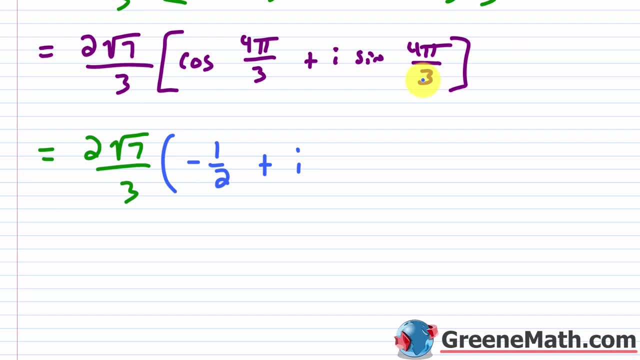 degree reference angle. we know that it's going to be in quadrant 3. sine is negative. so let me just go ahead and make that minus and basically pi over 3. the sine of that is going to be square root of 3 over 2, right? So it's the negative of the square root of 3 over 2.. Put the i out in front like this: 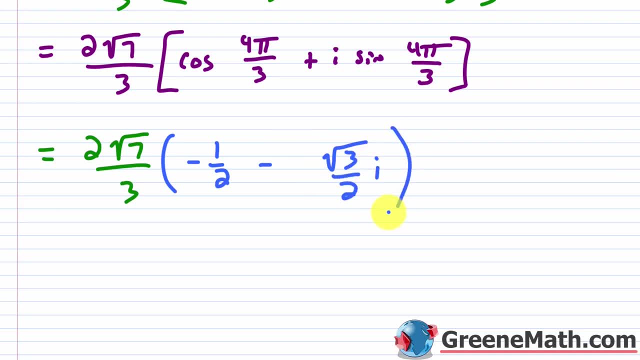 or typically with this situation. I'll put it here. so we'll close that down now And all I need to do is just distribute this inside to each term, right? So basically, I have 2 times square root of 7 over 3 times negative one half and then minus you'll have 2 times square. 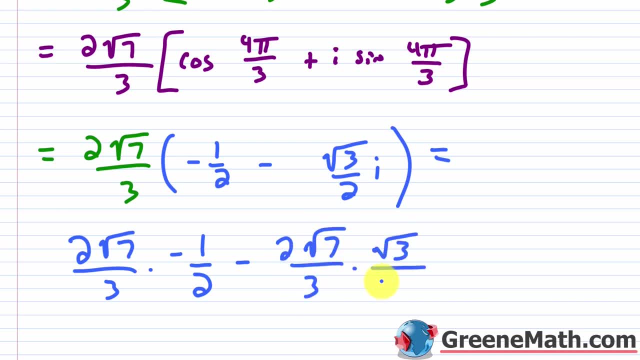 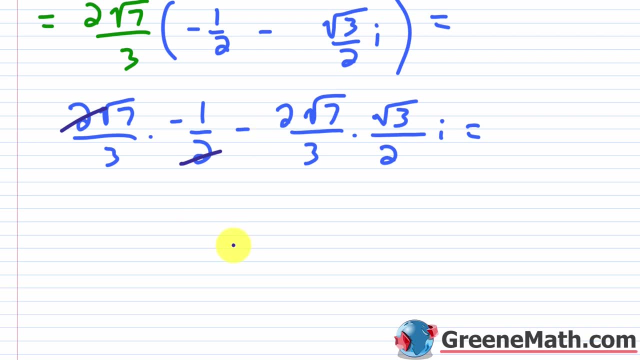 root of 7 over 3 times. square root of 3 over 2 times i. Okay, so let's come down here and just simplify and we'll have our rectangular form. So the 2's are going to cancel here. You'll have the. 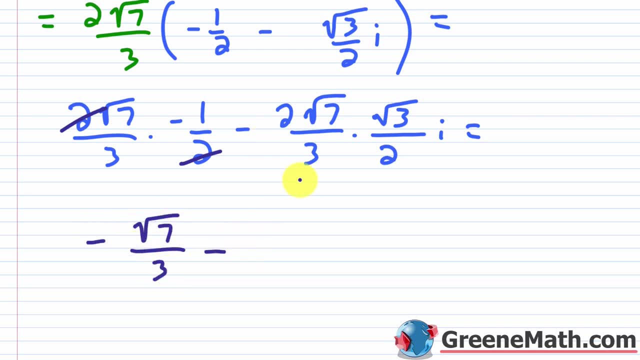 negative of the square root of 7 over 3 and then minus the 2's, are going to cancel here. Square root of 7 times square root of 3 is the square root of 2.. So that's going to be in quadrant 3.. 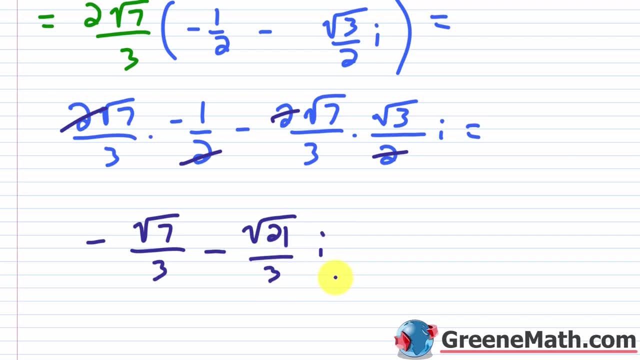 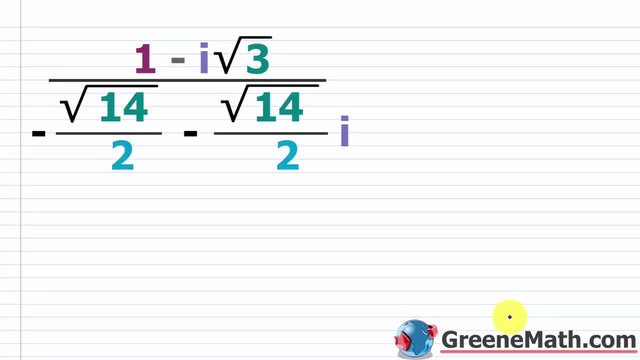 So you'll notice that this division here involves these two complex numbers in rectangular form. So what we're going to do is we're going to put these into polar form, We're going to use our quotient theorem and we'll just leave our answer in polar form. Okay, so let's start out by converting. 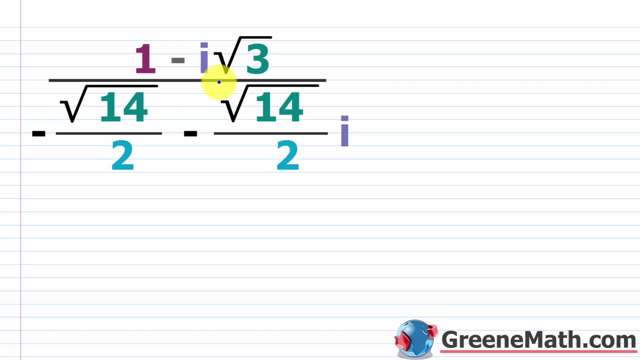 each one of these over. So I have 1 minus i times square root of 3.. I'm just going to do this on a separate page. So 1 minus i times square root of 3.. So the real part is 1.. The imaginary part is: 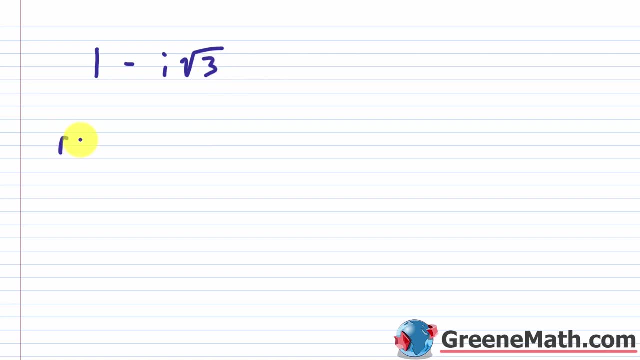 the negative of the square root of 3.. Okay, so let's go ahead and say my r is going to be the square root of 1 squared, which is 1, plus the negative of the square root of 3 squared, which is 3.. Okay so, let's go ahead and convert each one of these over, So I have 1 minus i times square. 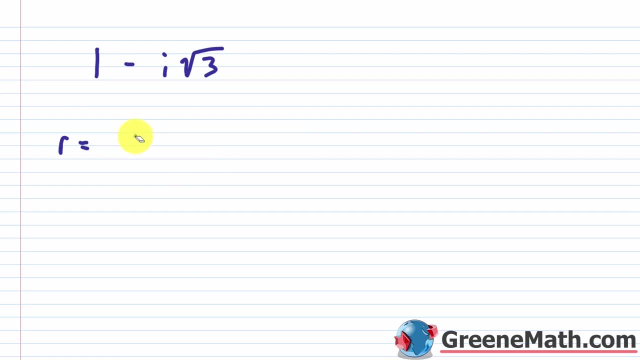 root of 3 squared. So obviously this is 4 and the square root of 4 is going to be 2.. Okay, so let's put this as 2.. Okay, so now I need to find my theta Right. so my argument for this guy, And so. 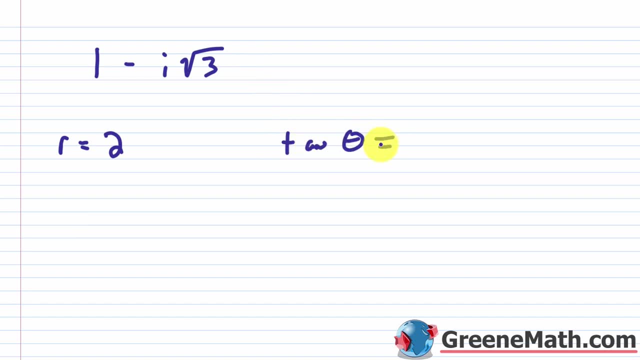 the tangent. the tangent of theta is going to be equal to the negative of the square root of 3 over 1.. Okay, might as well just say it's the negative of the square root of 3.. So let me go ahead and do the inverse tangent function. Okay, with the square root of 3.. Forget about the negative. 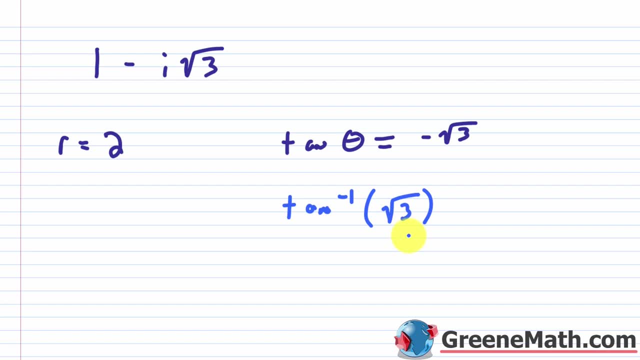 Punch that into the calculator. So what you're going to get there is 60 degrees or pi over 3. if you want to work with radians, Let's work with radians, since we work with degrees for the multiplication examples. So I'm going to say this is pi over 3.. Or you can just put 60 degrees if 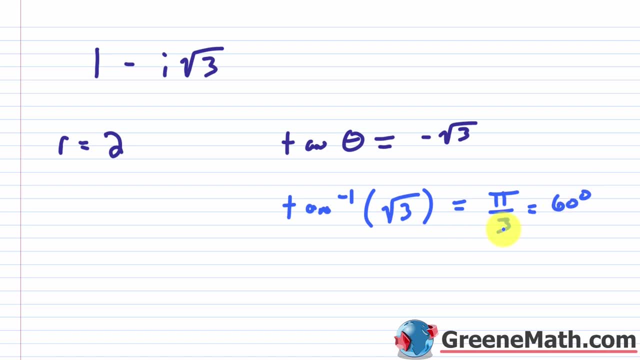 you like working with degrees, Okay, so let's put that there. Now, this is going to be my reference angle. Let's think about this guy. The real part here is positive, So I'm going to the right, And then the imaginary part here is negative, So I'm going down Right, so I'm going to the right, and 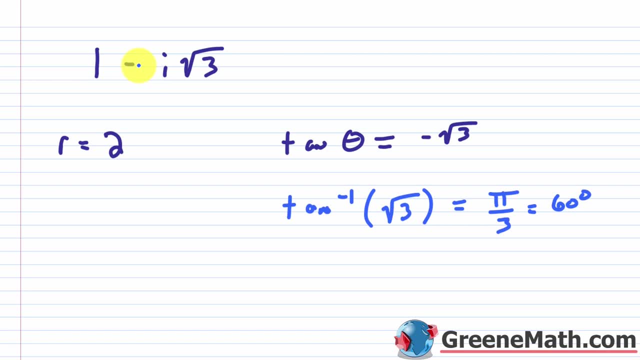 that means I'm going to be in quadrant 4.. So what I'd want to do is I'd want to subtract 2 pi minus this pi over 3.. Okay, to figure out what my theta is going to be. Okay, you can write this as 6 pi. 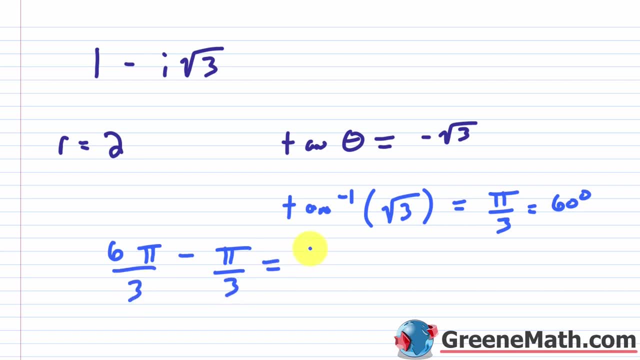 over 3.. So 6 pi over 3. And this is going to give me 5 pi over 3.. Okay again, if you wanted to do this with degrees, you do 360 degrees minus 60 degrees, you would get 300 degrees. So, however, 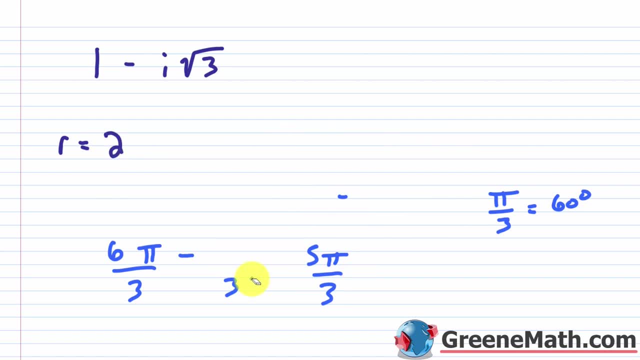 you want to do that, So let's go ahead and write this, since we have all the required information. I'm just going to say theta here. Theta is 5 pi over 3.. Okay, so in polar form we know that this is 2 multiplied by the cosine of this 5 pi over 3.. And then plus i times the sine of our 5 pi over. 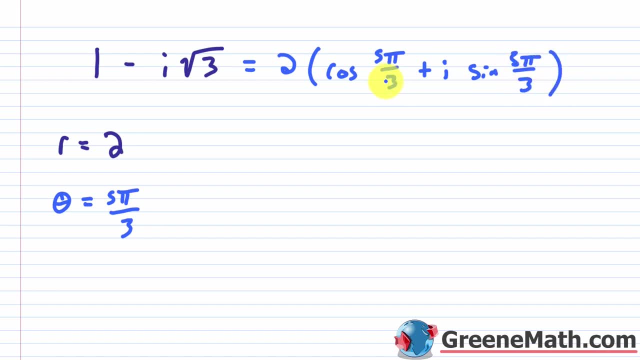 3. Okay again, if you want to put 300 degrees in there, feel free. Okay, so I'm going to get rid of this. Let's go ahead and look at the other one. So we have this negative of the square root of 14. 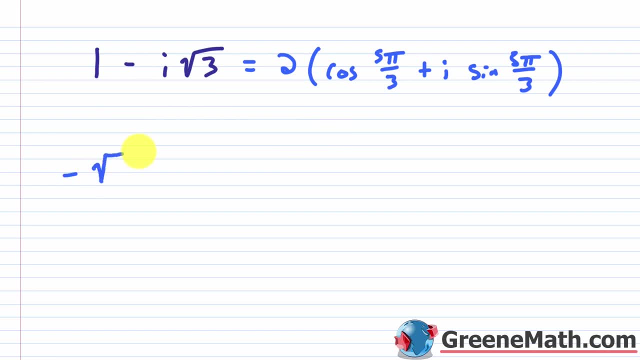 times i. So let's go back So we have the negative of the square root of 14 over 2.. Okay then minus. Let me put this down here so it's a little bit more consistent. We have this square root of 14 over 2 times i, So my r is going to be equal to the square root of. I'm going to take. 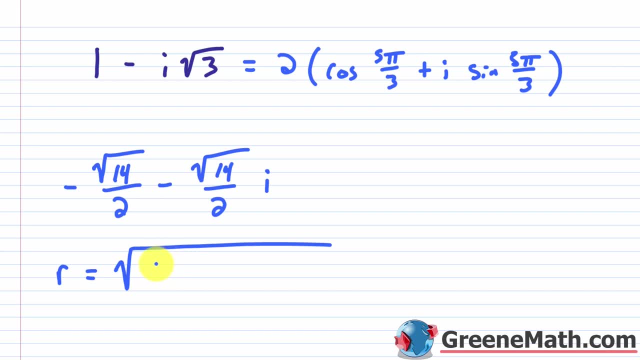 this guy. So it's negative in each case. Just forget about it. We're going to be squaring it. Let's go ahead and say it's the square root of 14 over 2 squared. Well, if I square the square root, 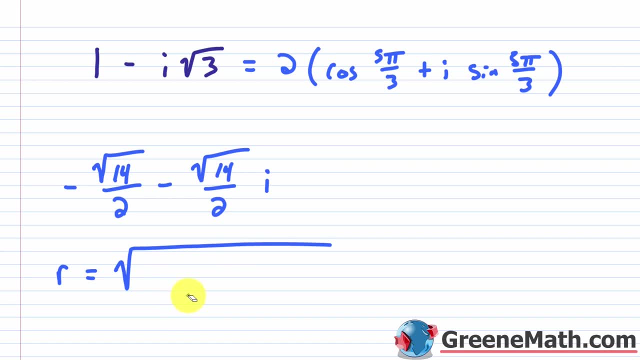 so this is going to end up giving me 14 over 4.. Okay, so 14 over 4, which is going to be 7 over 2.. So you would have 7 over 2.. Okay, plus 7 over 2.. Okay, so this would end up giving me 14 over 2. 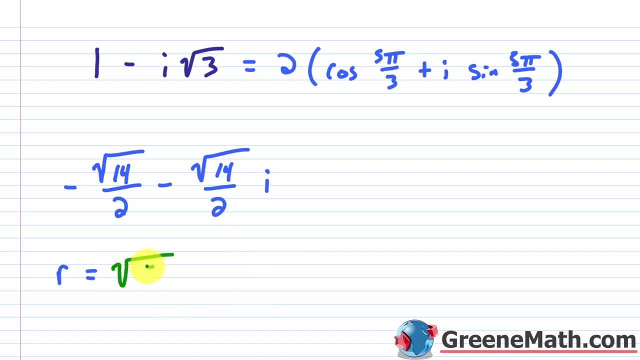 which is 7.. Okay, so this will be the square root of 7.. Okay, so that's all that is. So that's my r value. Let me drag this up here, so it's out of the way. So now let's figure out what is the theta. 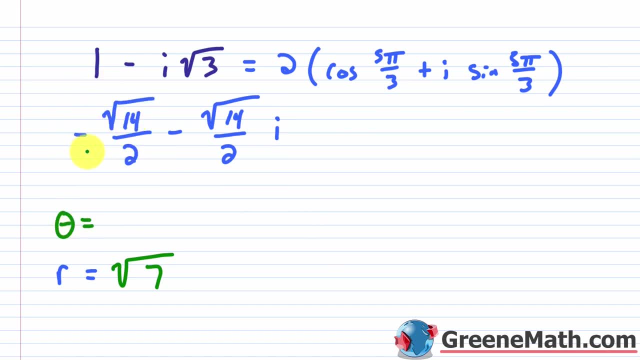 Okay. so again, if you look at the square root of 7.. Okay, so, that's the square root of 7.. Okay, so that's the real part and the imaginary part. In each case, it's the same thing, Right? so if I did tangent, 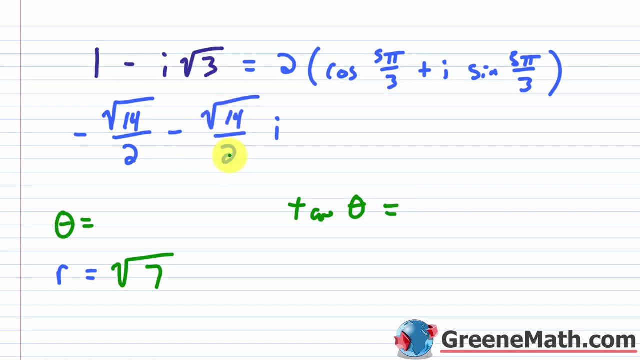 of theta is equal to: if you did the negative of the square root of 14 over 2, then over the negative of the square root of 14 over 2, that's just going to end up being 1.. Okay, so if I did the tangent, 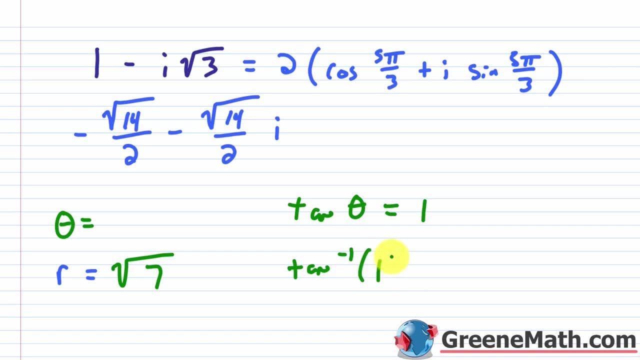 the tangent inverse of this guy of 1, I get 45 degrees, or in terms of radians it's going to be pi over 4.. Okay, so you can put that, or you put 45 degrees, whatever you want to do So for this guy. 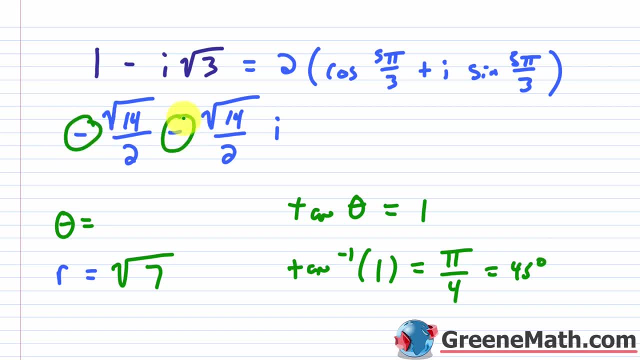 this is negative of 14 over 2.. Okay, so if I did, the tangent of theta is equal to, if you did, the tangent inverse of this guy of 12. you can put that, or you put 45 degrees, or, in terms of radians, Bye, and this is negative. So I'm in quadrant 3 and I'm going to the left and I'm going down. 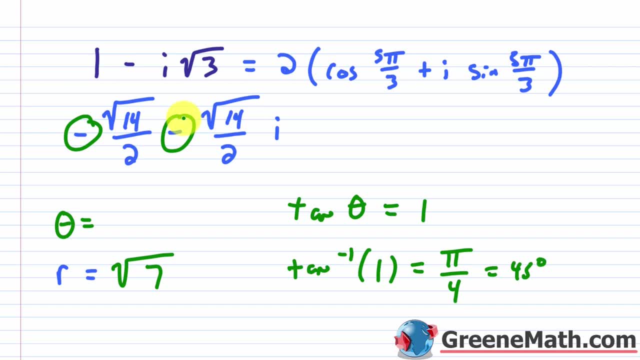 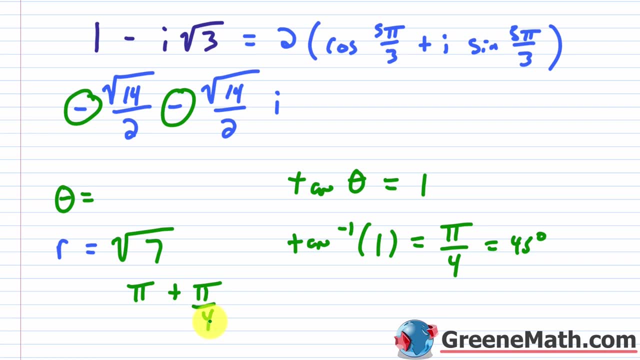 So in quadrant three I would want to take pi and I want to add pi over 4 to get that angle. so pi plus pi over 4, or again you could do 180 degrees plus 45 degrees, whatever you want to do, Okay. so for this one, I'm going to multiply this by four over four. 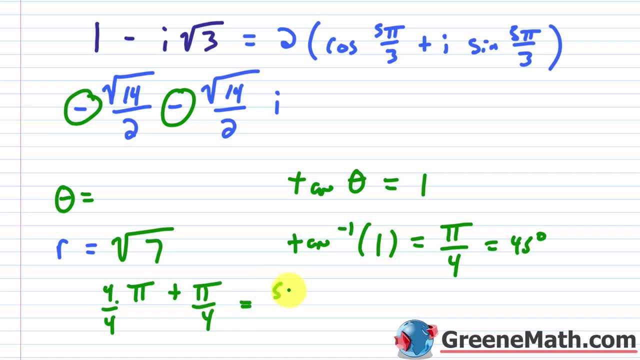 so this will end up being 4 pi plus pi, which is five pi, and then over the common denominator of four. I'm an ideal, benevolent theorem and an intelligent phenomenon. butnost söz to ycar déดолог. perfectly fine, because it's completed, because it's 51 degrees by 45 in from × The. 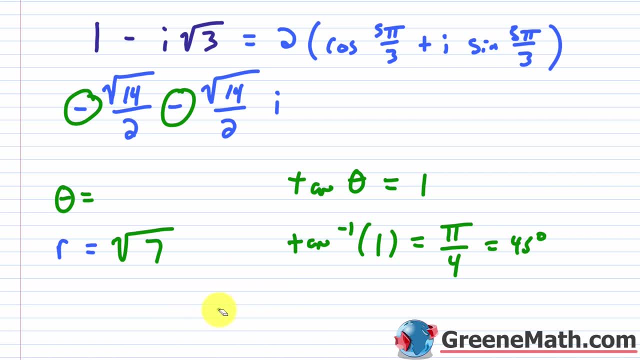 So this is 5 pi over 4, or 225 degrees if you're working with degrees. So let's put 5 pi over 4 like this. let's get rid of all this. So in polar form this guy is going to be, we have our square root of 7, multiplied by 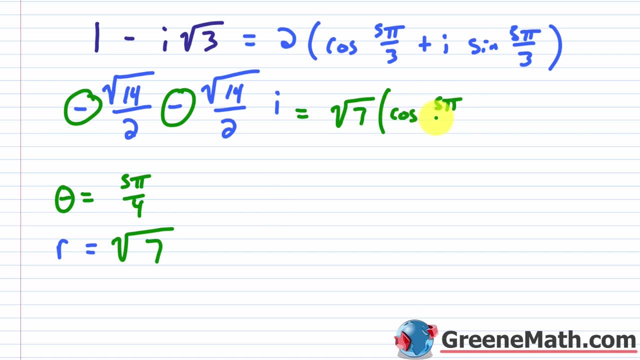 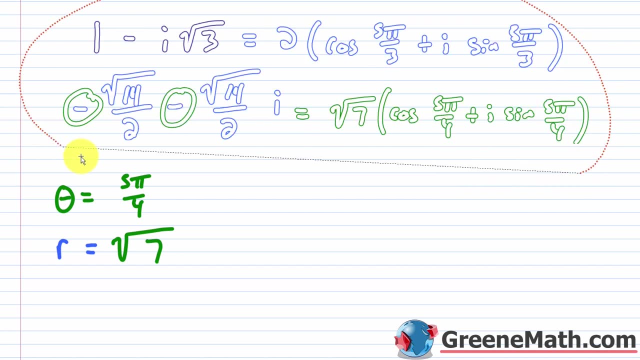 we're going to have our cosine of 5 pi over 4,, plus i times the sine of 5 pi over 4, okay, So this part's done. let me copy this. let's come back up to our problem. paste this in: 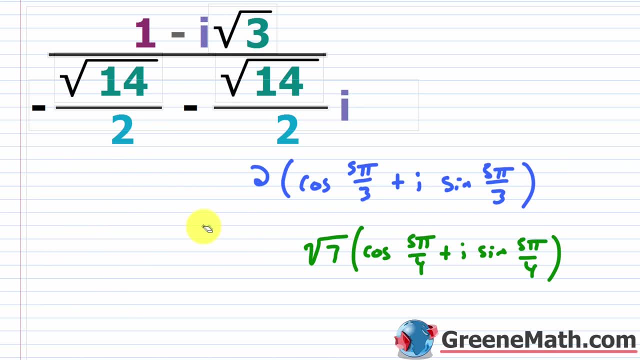 real quick And I'm just going to get rid of this and what I'm going to do is I'm going to put equals like this, and I'll just drag this over and I missed something, so let me get all of this. 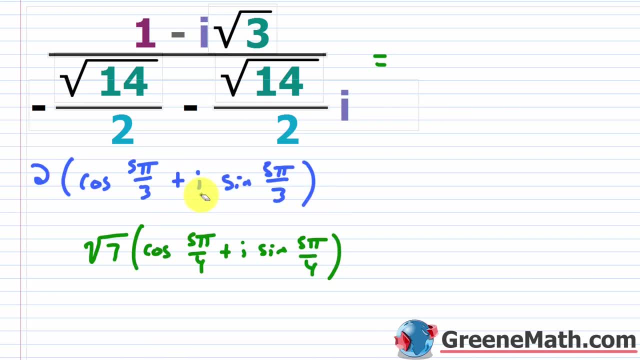 drag this over here. let me put my little division bar, and I did that terribly, so let me try that one more time, And let me just scooch this down just a little bit, so it lines up perfectly. alright, there we go. 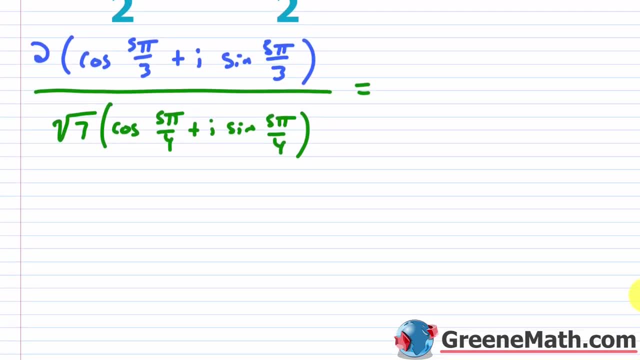 So now what I want to do is just use my quotient theorem. okay, very easy at this point. So 2 divided by the square root of 7,. so 2 divided by the square root of 7, of course, you can rationalize the denominator. 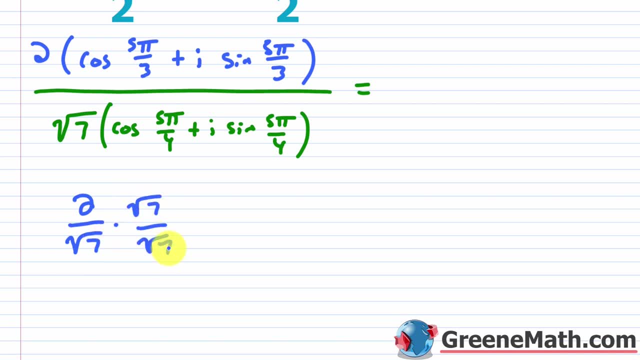 I can multiply this by the square root of 7 over the square root of 7.. So this is 2 times the square root of 7 over 7, so 2 times the square root of 7 over 7, so that's that part, that's done. 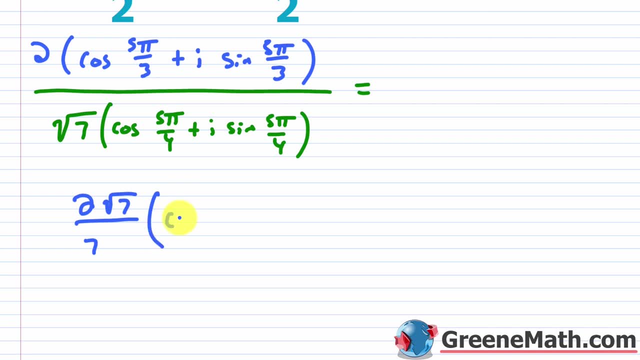 And then, basically, what we want to do, times this quantity. here you have the cosine of. you're going to have 5 pi over 3, minus 5 pi over 4.. And I'm making this terribly, so let me kind of edit this a little bit. so this is a 5. 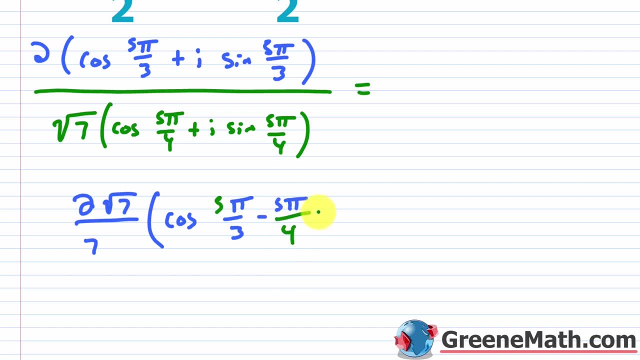 and this is a 4.. And of course, we need a common denominator. Let's just stop and get this. So we need to go 3 and then 3, we need to go 4 and then 4.. So this would be 20 pi over 12,. this would be 20 pi over 12, minus it would be 15 pi. 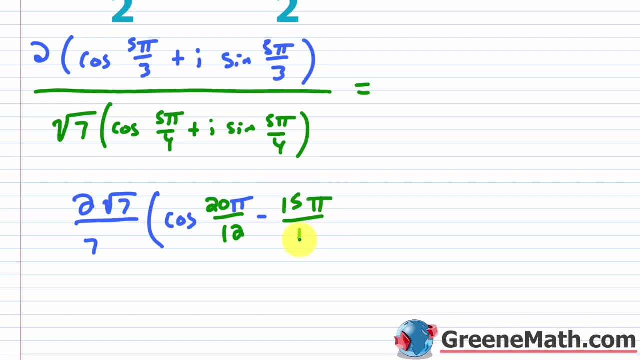 over 12.. So 15 pi over 12,. okay, So this would give me what It would give me: 5 pi over 12.. So the cosine here of 5 pi, 5 pi over 12.. Then I'm going to have, plus, I have my, i times the sine of: again, it's the same thing. 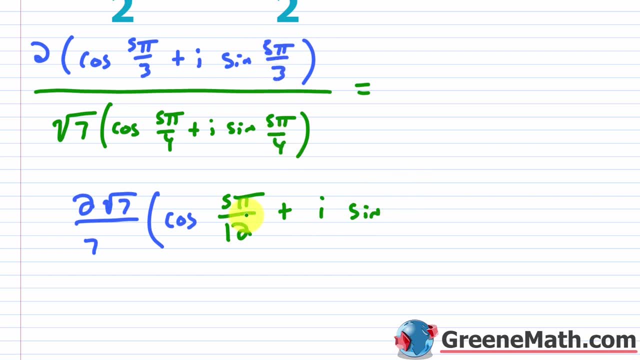 So the 5 pi over 3 minus the 5 pi over 4.. So that gives us the 5 pi over 12.. So this is going to be our result in polar form. Again, if you wanted to figure this out in rectangular form, just evaluate the cosine. 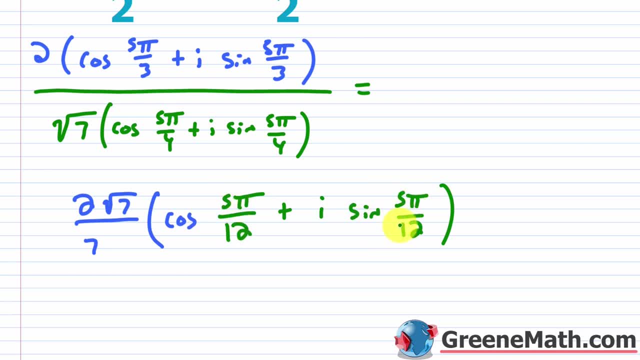 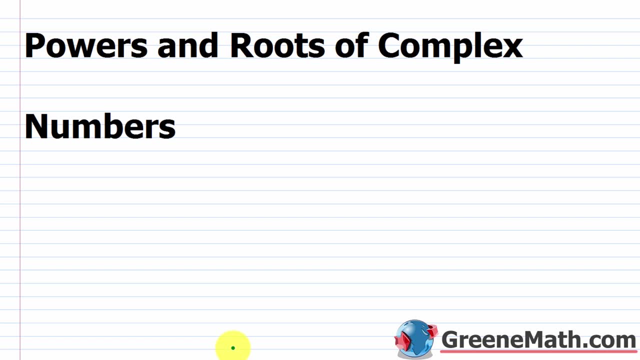 of 5 pi over 12, evaluate the sine of 5 pi over 12, get those values and then just use your distributive property here to set that guy up. In this lesson we want to talk about powers and roots of complex numbers. 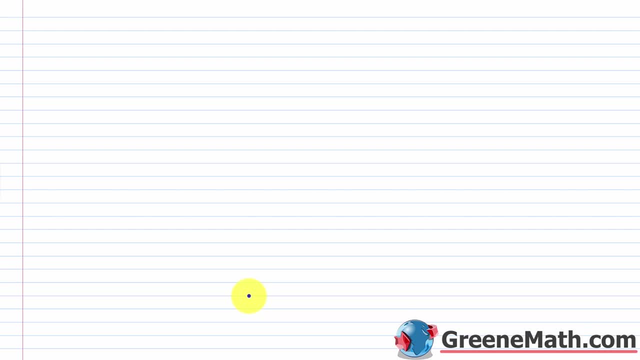 Alright. So in the last lesson we talked about multiplying two complex numbers together when they're in polar form, using something called the product theorem. So what we're going to do here is just go a step further and we'll talk about these powers and roots of complex numbers. 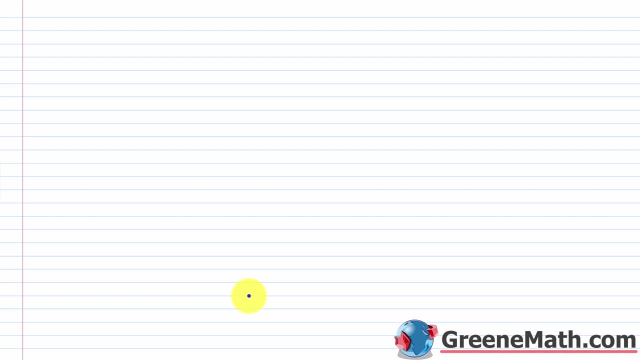 So what I'm going to do is I'm just going to start out with a simple, complex number, something generic in polar form. So I'm just going to write: r times the quantity cosine of theta, plus i times the sine of theta. Okay, 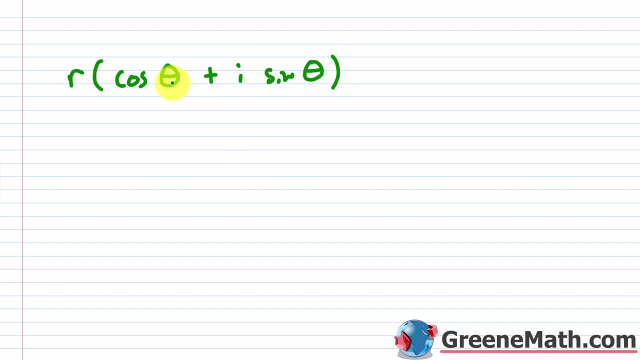 So when we talk about r, that's the absolute value of the complex number. When we talk about theta, it's referred to as an argument. If you think about the complex number as a vector, it's going to be the direction angle. 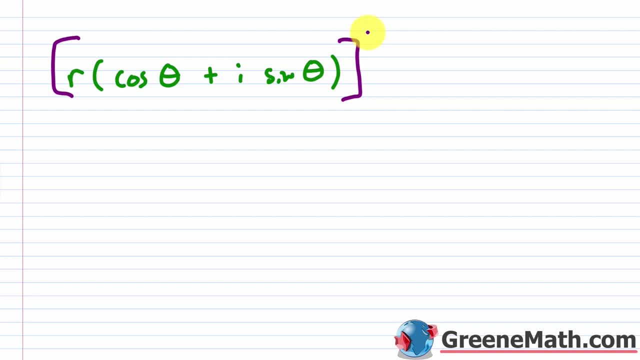 So let's say that I wanted to raise this to, let's say, the second power. So I'm squaring this and basically what I would do here. I would just expand this. So this would be r times the quantity of the cosine of theta, plus i times the sine of theta. 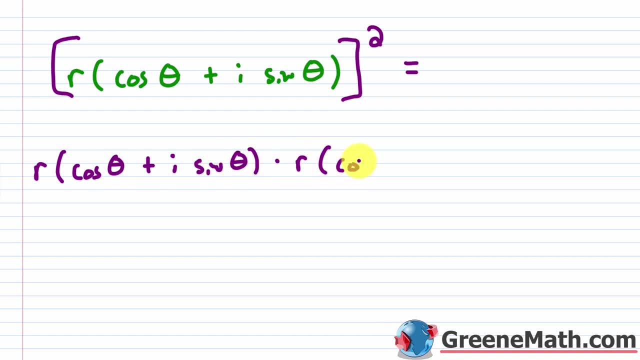 And I'm going to multiply by itself. So r times the quantity of the cosine of theta. So you can see here that you have r times r. Remember you're multiplying the absolute values together. So this gives me r squared. Notice that this guy right here, this exponent here on r, matches this exponent here. 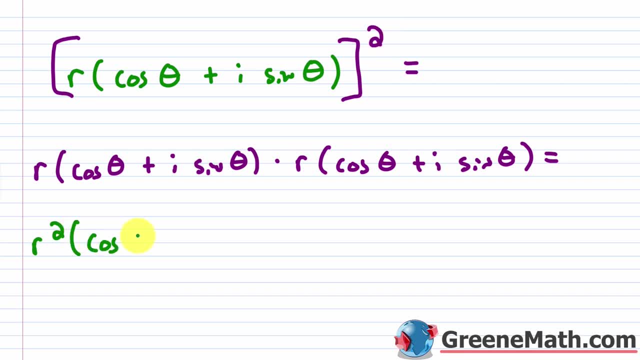 Okay, So this is going to be important. Then times the quantity you have cosine of, remember, you add the arguments. So theta plus theta is 2 theta. Then plus i, times the sine of theta plus theta, You add the arguments. 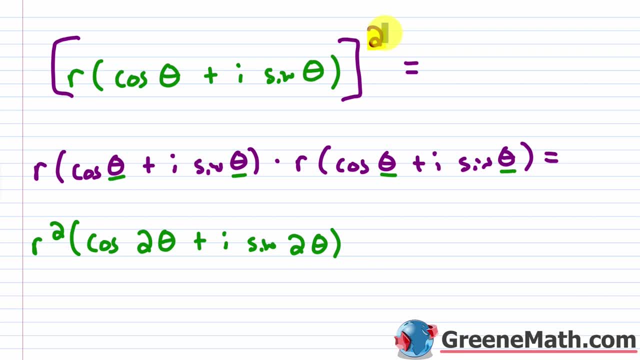 This is 2 theta. So I want you to notice some things Again, this 2 here, this exponent matches this exponent here, And then this guy here inside the parentheses, it's multiplying the argument. So the general rule is: whatever this exponent is- and this can be any real number- 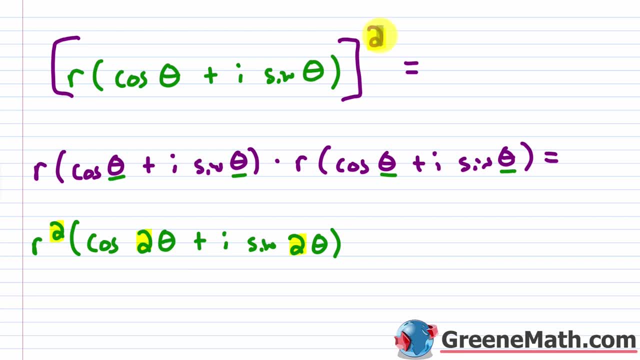 For today, we're just going to work with positive integers. But whatever this guy is, it's going to basically be your exponent on r, And then it's going to be multiplied by your argument inside the parentheses. Okay, Now I can do another one with you, just to show you this. 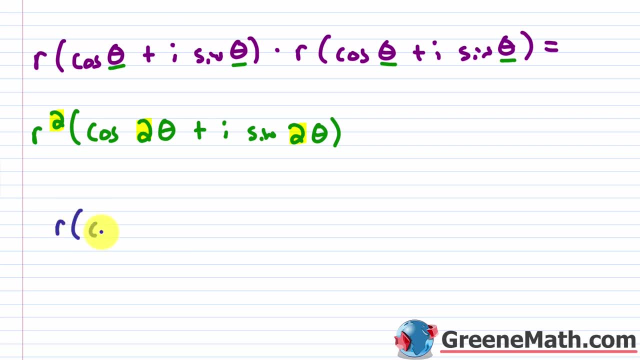 So let's say we did Something like r times the quantity cosine of theta, plus i times the sine of theta. Okay, Let's say now we cube this guy. Okay, So we know that this would be equal to basically this guy times this guy times another one. 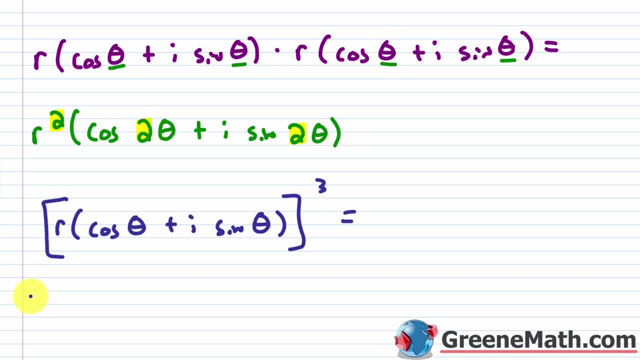 Okay, This guy times this guy. would give me this guy, So I can go ahead and write: r squared times the quantity cosine of 2 theta plus i times the sine of 2 theta. Okay, Then, multiplied by one more of these So r times the quantity cosine of theta plus i times the sine of 2 theta. 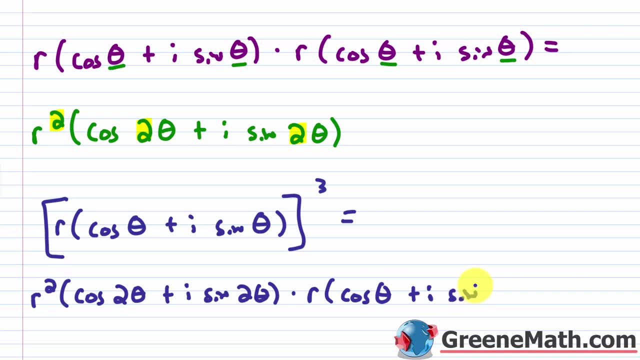 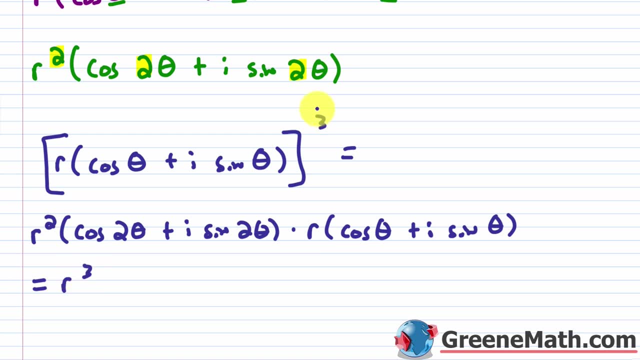 Okay. So what is this going to give me? Again, r squared times r is going to be r cubed, So r cubed Again. notice: this exponent here matches this exponent here. Okay, So basically, after that, inside the parentheses, you're going to have the cosine of 2 theta. 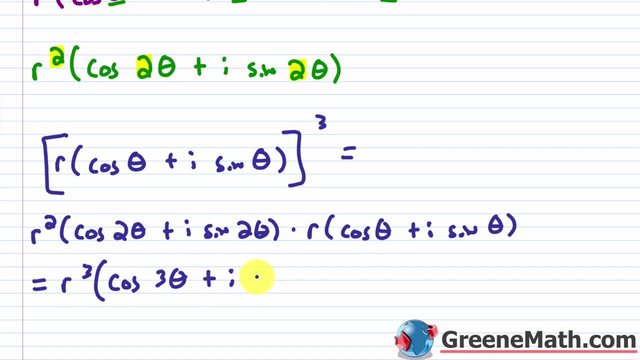 plus theta is going to be 3 theta. Okay, Plus i times the sine of 2 theta plus theta is 3 theta. So again, this exponent here of 3 is going to be You're exponent over here. I'm not going to write a 1, 2 of anything. 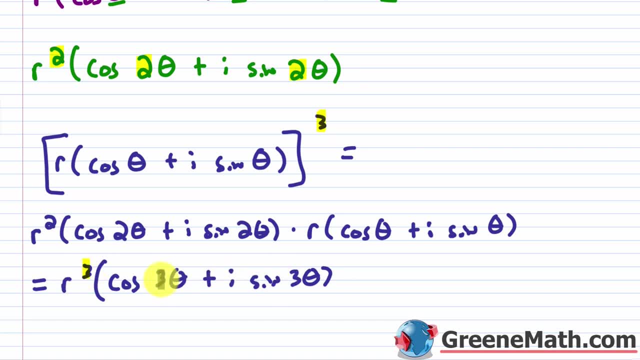 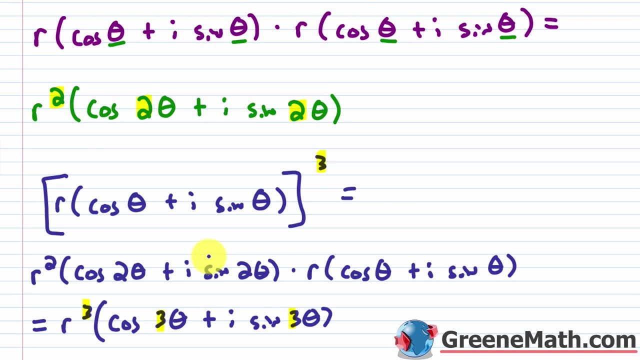 Okay, here on r and then inside the parentheses, is going to be multiplying your argument. okay, and this should make sense, because if i'm raising this to the third power, i'm cubing this. then basically i have three of these, so i have one, two and then a third one, right? so it makes sense that. 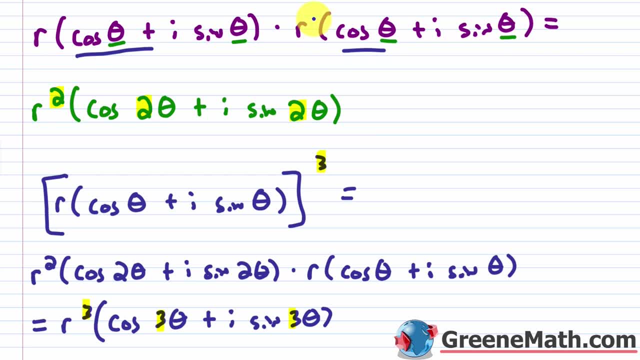 i have one, two, three r's, so it's going to be r cubed right, r times r times r, and then you have this one, this one and another one. so if you're adding the arguments, you have theta plus theta plus theta, which is three theta. okay, so that's what's going to work. if you raise this to the 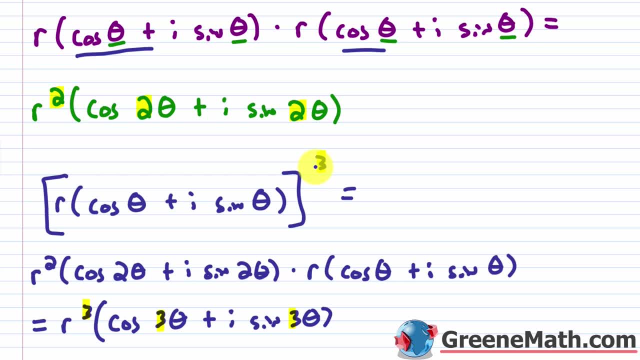 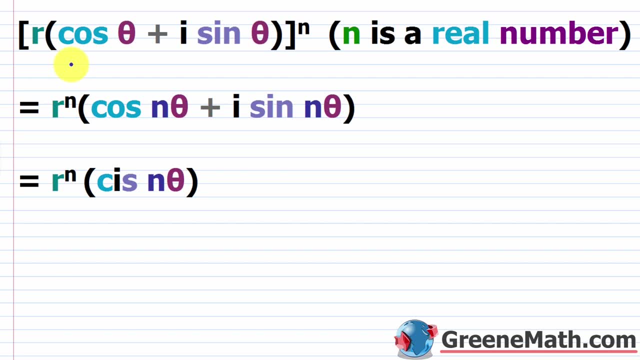 fourth power. you see the same thing. fifth power, sixth power, whatever you want to do, any real number, okay. so formally, this is our theorem here. you can write this down for your notes. basically, if you have some complex number in polar form, so let's say r times the quantity cosine of theta. 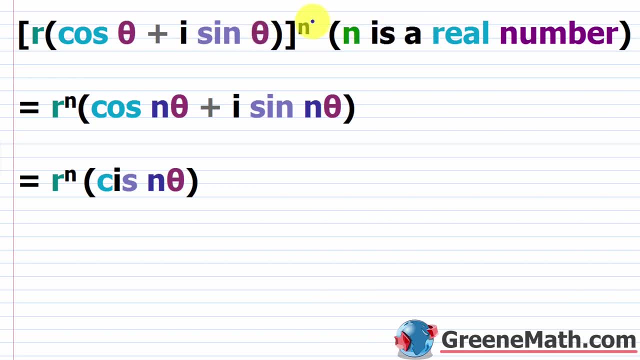 plus i times the sine of theta, and this is raised to some real number. n okay, again, we're going to use just positive integers today. then basically you can say: it's r to the power of n times the quantity you have, cosine of n times theta, plus i times sine of n times theta. okay, so this n is. 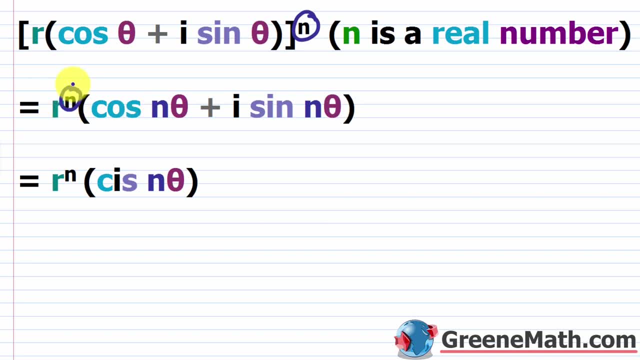 going to be multiplying your argument and it's also going to be your exponent on r, with the absolute value of that complex number. again, for the shorthand, remember this is the c, the i, the s. that's where this abbreviation comes from. so we have r to the power of n, and then you have this cis, the cis, some people say. and then we have 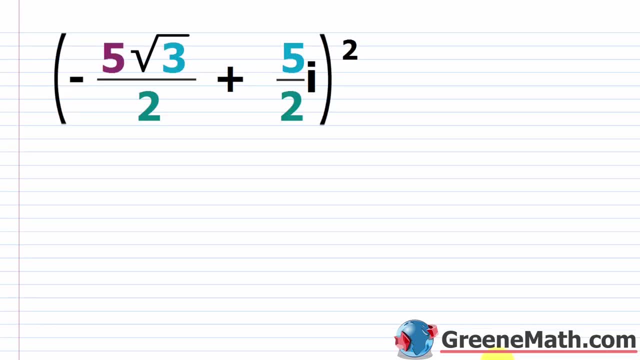 n times theta. all right, let's jump in and look at an example. so we're going to start with something very, very easy. so we have the negative of five times square root of three over two plus five halves i, and this whole thing is being squared now. obviously, this is 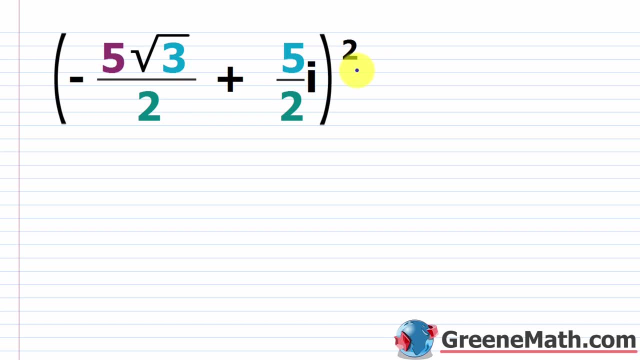 in rectangular form, and since this is just being squared, you could expand this and just perform the operation that way. but what we're going to do is use our little theorem. so we're going to first write this in polar form, then we'll use the theorem. okay, so i'll say this is equal to i'm. 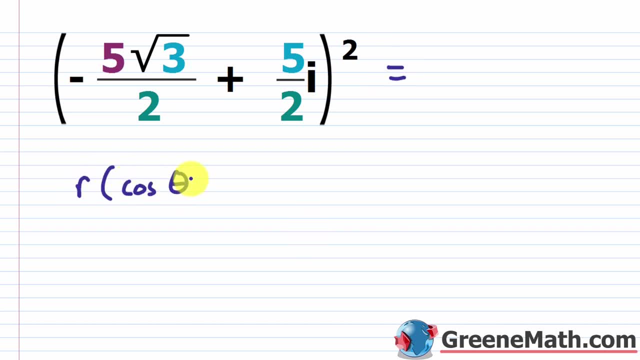 going to put my r times the quantity cosine of theta, plus i times the sine of theta. okay, and this is going to be squared, okay. so i'm going to fill out my r and my theta, so to get those, remember your r, okay, which is the absolute value of the complex number n, and then i'm going to put my r. 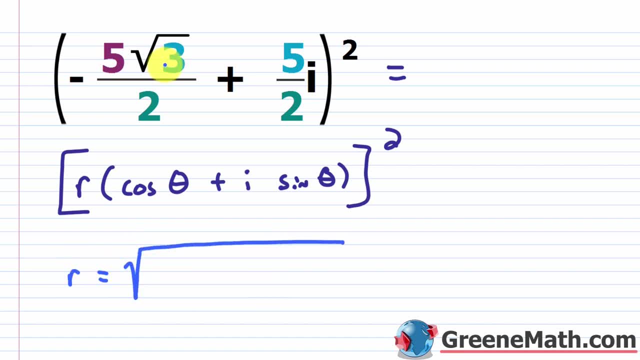 times the sine of theta and i'm going to 45, to the power of n, and when i add that up again I get like a pretty big square base. so you're going to realize that this multivariate number actually has that loss already, so that this both the minus 5 times square of thicc. 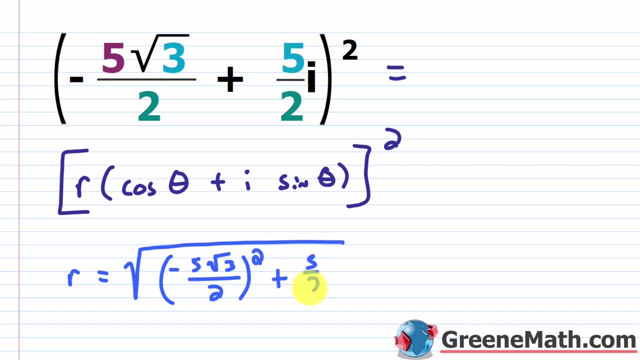 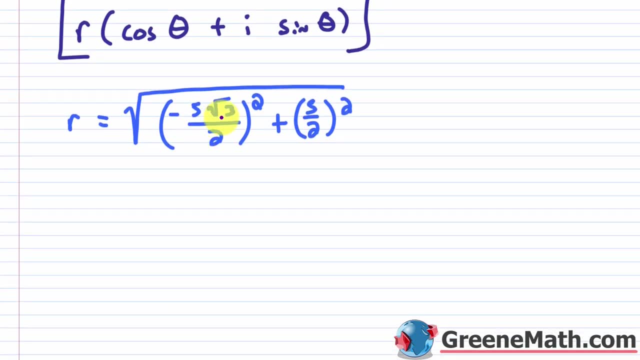 plus worked out. so if I analyze this with a, a square number, so if i overshoot this here, let's make sure that I do this here. given that I have this square root of n, lets make sure that this was in absolute square root of 3. i go into эта and it's going to. 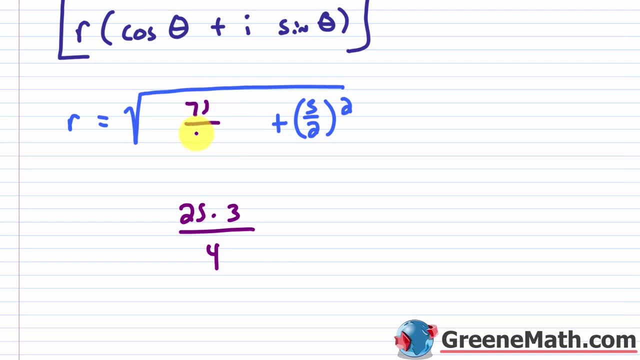 be just like a zero. Nothing's going to change here. I just have to go ahead and just make and put 75 over 4, and that is a terrible 5, so let's fix that. and then the 5 half squared is just 25 fourths, so let's put plus 25 fourths. now, 75 plus 25 is 100, and 100 divided by 4 is 25. 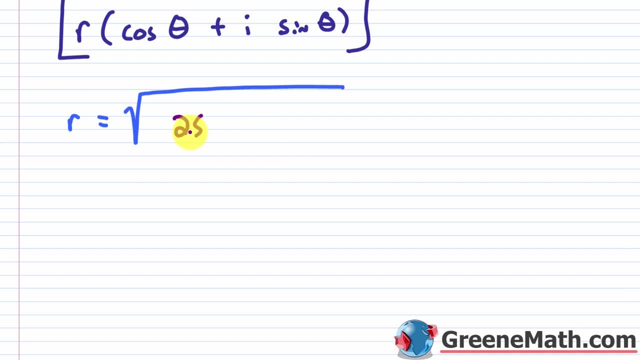 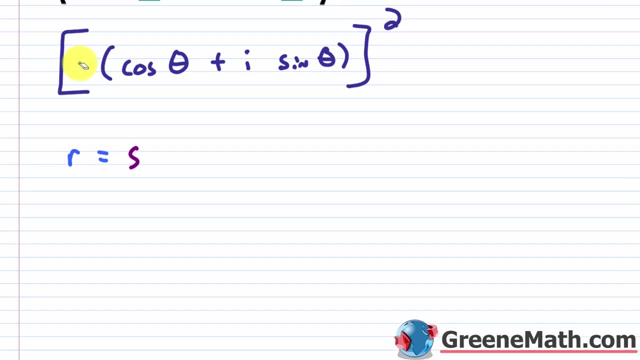 okay, and obviously 25 is a perfect square. square to 25 is 5, okay, so let's say this is 5. now let me come up here just a little bit, so let me scroll up just a little bit. i'm going to erase this r. 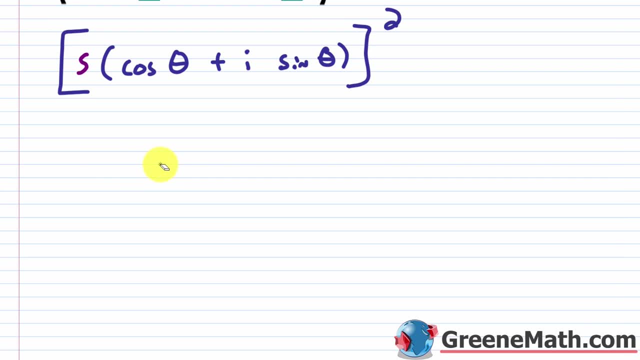 and i'm going to put a 5 in there for the actual value. and now i need to figure out what theta is. so lots of ways to think about this. remember your tangent of theta. if you're thinking about this as x plus y, i, well it's going to be y over x, okay. if you think about this as a plus vi, then 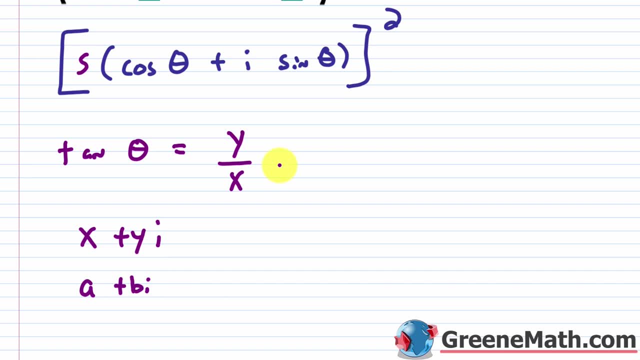 it's b over a, it's the imaginary part over the real part. okay, but you have to be careful about this, because when you use your inverse tangent function, you're only going to get something in quadrant one if this guy's positive, and something in quadrant four, rotating clockwise, if this guy's. 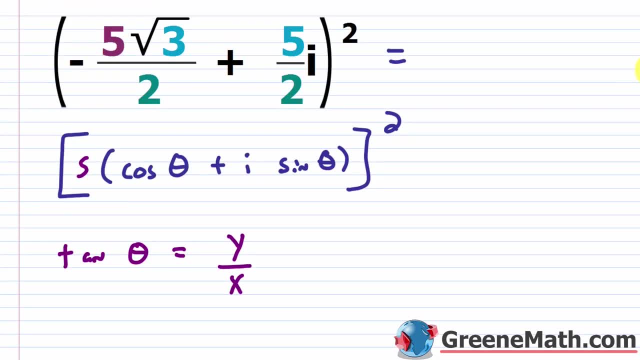 negative. okay, so you have to be real careful about this, because when you use your inverse tangent function, you have to be real careful here. so let's come up and think a little bit about this. so the y part is five halves. okay, so that's five halves. then i'm dividing by a fraction, so i'm 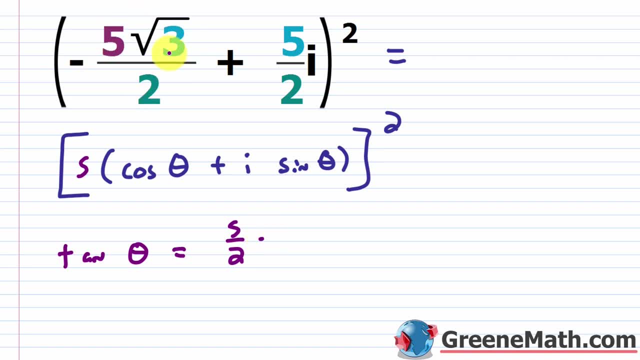 going to multiply by the reciprocal. the x part, or the real part, is going to be the negative of five times square root of three over two. i'm going to flip that, so i'm going to put two over five times square root of three. okay, i'm dividing fractions. that's why i did that. okay, so what i would see? 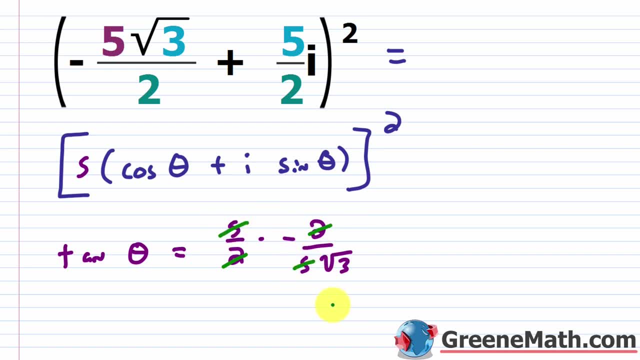 here is that this would cancel with this and this would cancel with this. so i have the negative of one over the square root of three. rationalize the denominator: this is square root of three over square root of three, and so this gives me the negative of: you have the square root of three. 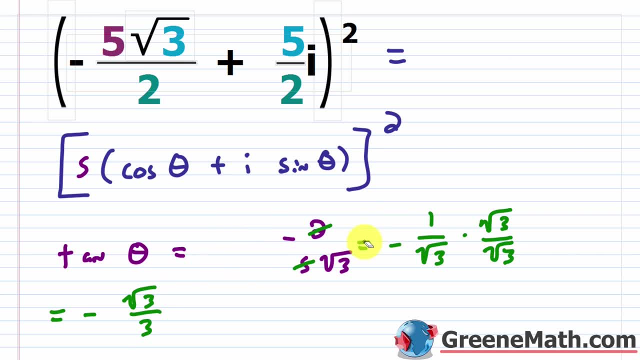 over three. okay, so let's think about this formula. if i type this into my calculator, okay, as the inverse tangent of this guy, i'm going to get something in quadrant four, and i'm also going to get a negative angle. okay, so it's going to rotate clockwise. that is not what i want, okay. 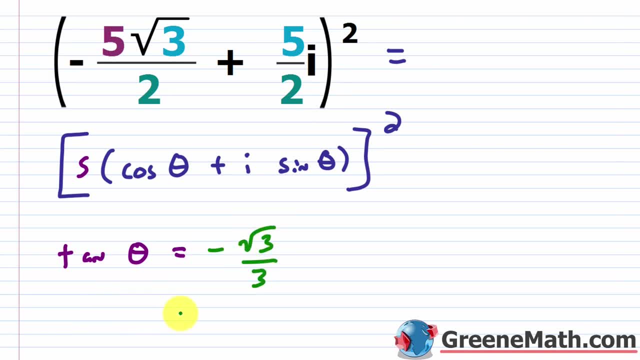 so what i'm going to actually do is i'm going to do the inverse tangent of. i'm just going to make this positive. so, square root of three over three. this is going to give me my reference angle, okay. so if i punch this into the calculator, i get pi over six. okay, if you want. 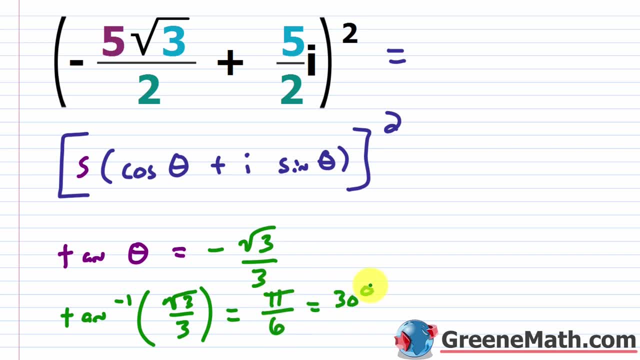 to work with radians, or you get 30 degrees if you want to work with degrees. now, this is not my answer, because i'm not in quadrant one. okay, let's get rid of this. we don't even need this anymore. okay, let's think about where we are. if you were to graph this complex number on the complex plane, 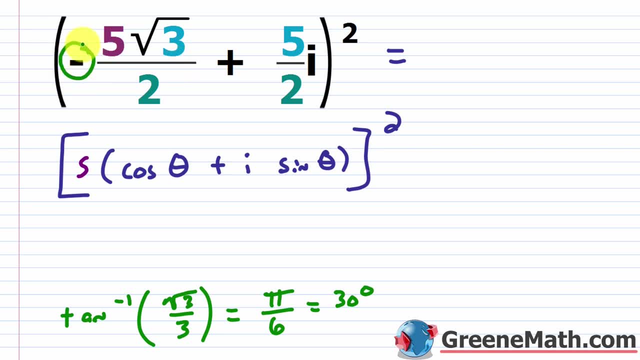 then, basically, you think about the fact that this is negative, so the real part's negative and this is positive. right, so this is positive. so from the origin i would go to the left and i would go up. that puts my complex number in quadrant two. okay, so in quadrant two i want an angle with a reference. 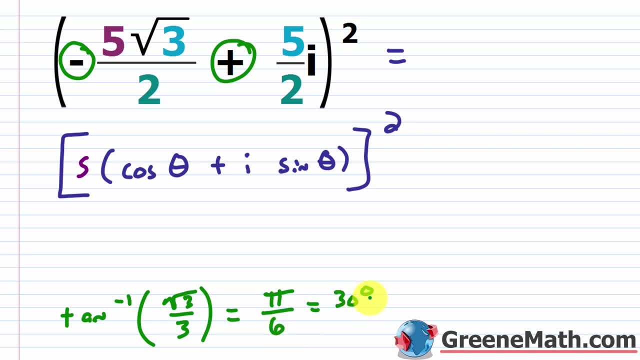 angle of pi over six or 30 degrees, okay. so basically you can say theta is equal to. you could do pi minus your pi over six. okay, and i can do six pi over six to get a common denominator. so this is five pi over six, which is 150 degrees, right? if you wanted to do this with degrees, you. 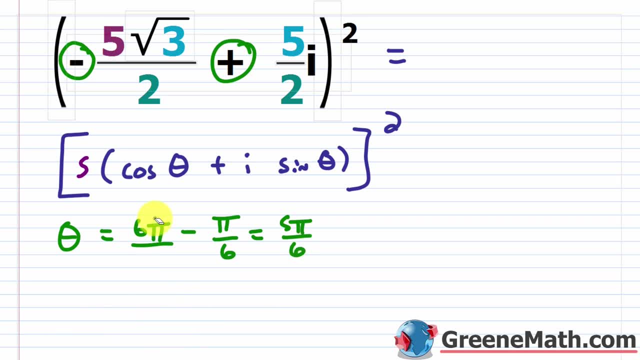 do 180 degrees minus 30 degrees. you could do this with degrees: you do 180 degrees minus 30 degrees, so again it's 150 degrees. so let's do five pi over six. so five pi, pi, pi over six. so that's the tedious part. so let's just erase this and this and go five pi over six. of course you can put 150 degrees in. 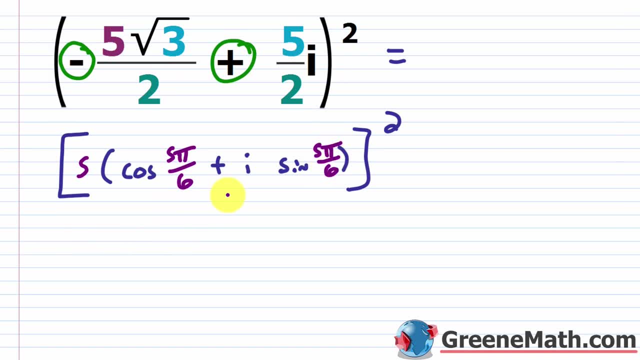 there. if you feel more comfortable with that, that's up to you, okay. so now that we have this done, finding our result here is really easy, right? using our little theorem, this r value here is raised to this power. so five is squared, five squared is 25. that's easy, then times five is: 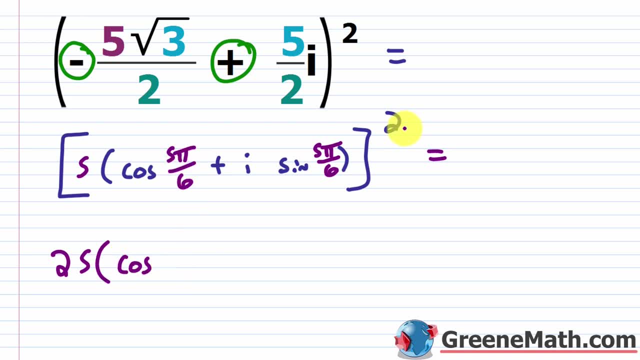 squared times the quantity. the cosine of this gets multiplied by this exponent, so we'll have- let me do this in a different color- two times five pi over six. okay, then plus let me return to this other color. so, plus your, i times the sine of: again, it's going to be two times five pi over six, okay. 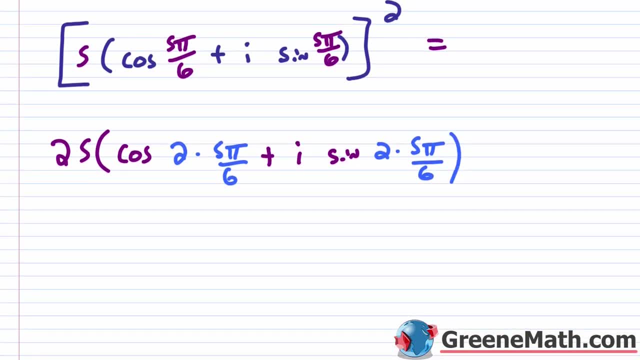 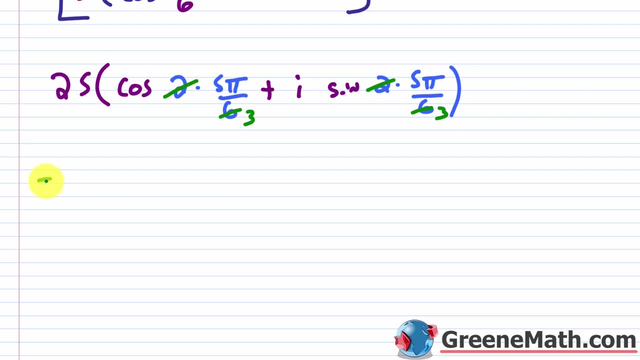 that's all it is. it's very, very simple. most of the work is just putting it in polar form, so once we have this we can think about: okay, well, this would cancel with this and give me a three. this is going to be 25 times a quantity. you have your cosine of five pi over three. okay, plus i times the. 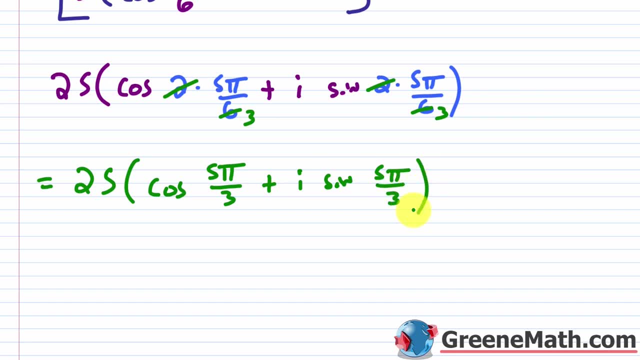 sine of five pi over three. okay, and five pi over three is 300 degrees. if you want to write it like that, again, up to you. now, this is the answer in polar form. if you want to put it in rectangular form, again, it's all over the place in terms of what your teacher would ask for. let's just get a. 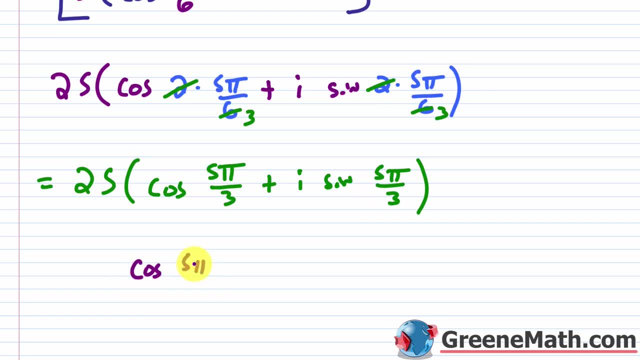 little quick practice with that. so the cosine of five pi over six is going to be three times five pi over three. again, the reference angle there is pi over three, okay, or 60 degrees. so the cosine of pi over three is going to be a half right and cosine in quadrant four is going to be positive. 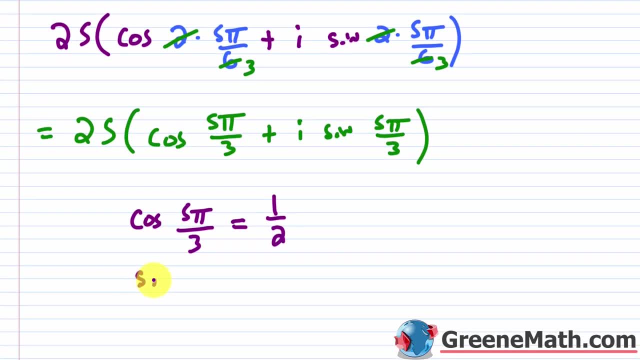 so this equals one half, now the sine of five. pi over three, again pi over three. if you think about the sine of pi over three, well, that's going to be square root of three over two, but we're in quadrant four, so this is the negative of the square root of three over two. okay, so let's go ahead and replace. 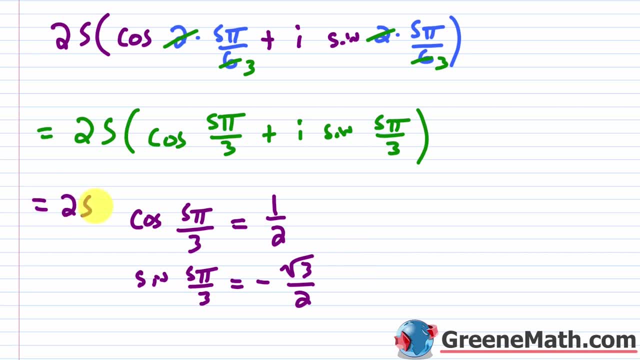 these. i'll go ahead and say this is equal to 25 times. i'll say this is one half, so this is going to be one half, and then plus you have, i multiplied by this is going to be the negative of the square root of three over two. probably better to kind of switch this around here and then maybe scooch. 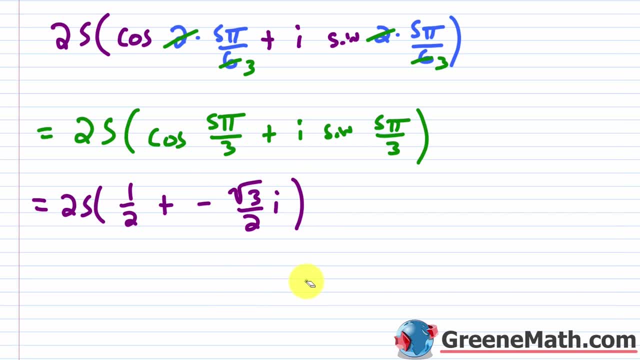 this down a little bit for formatting and let's close this down. okay. so let's go ahead and distribute this 25 in, so this is the negative of the square root of three over two, and then would be 25 over 2, and then basically I have plus negative here. might as well just write minus, it's. 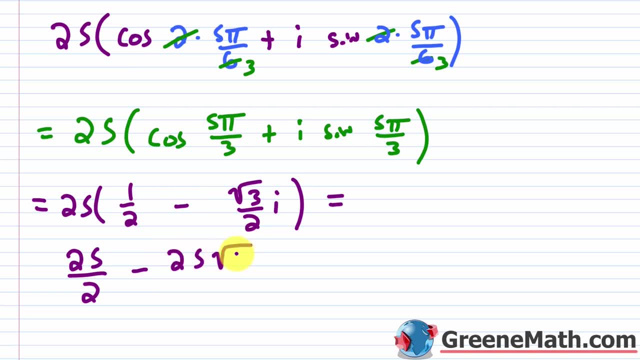 a little bit easier. I'll say minus 25 times square root of 3 over 2. now you can put your i out here and then sometimes people put the i there. it's really up to you. it's very clear here that it's not under the square root symbol, so I would just leave it like this. so this would be your answer. 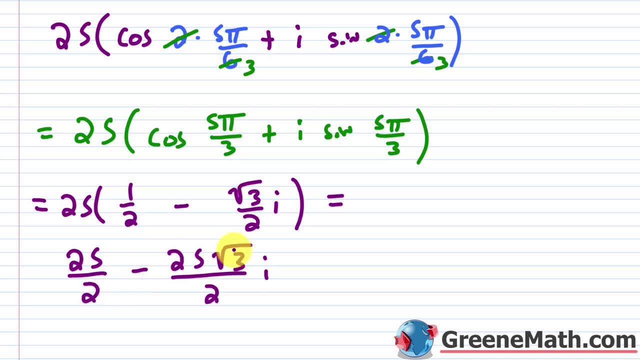 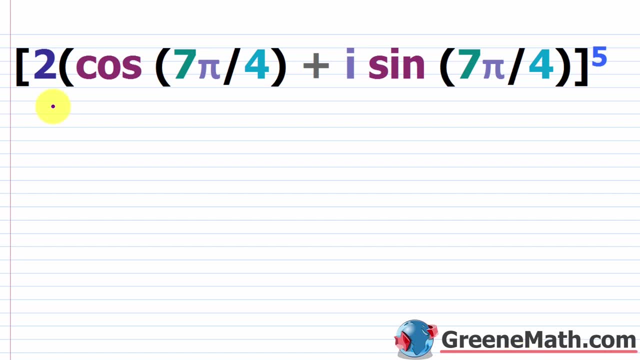 in rectangular form, your 25 over 2, minus 25 times square root of 3 over 2, and then times i. all right, let's look at another example. so this one, I'm going to give it to you in polar form, make it a little bit quicker. so we have 2 multiplied by the quantity cosine of 7 pi over 4 plus i times. 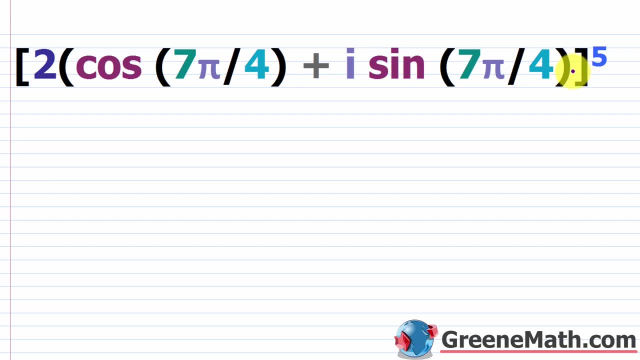 the sine of 7 pi over 4 and this whole thing is raised to the fifth power. okay, so if it's in polar form already, it's super easy, right? this r value here, this 2, is going to be raised to the fifth power. so you have 2 to the fifth power. we know that's 32. we'll just simplify that in a moment. 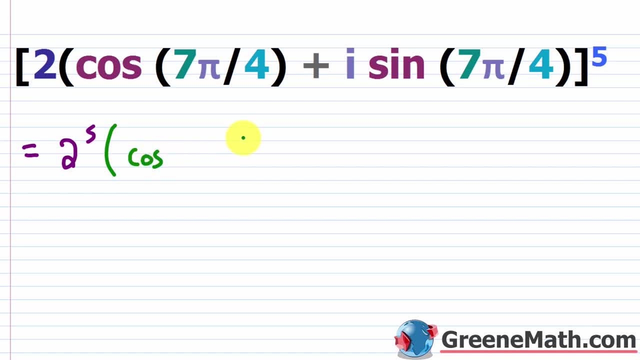 then inside the parentheses you'll have your cosine of again. this x is going to be raised to the fifth power, so you have 2 to the fifth power. exponent here of 5 is going to be multiplied by the argument. So 5 times 7, pi over 4, okay. 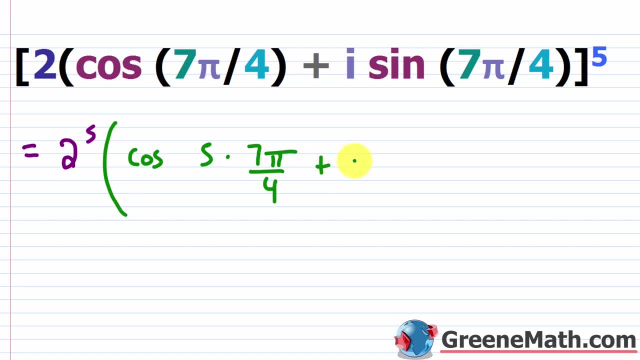 maybe make these parentheses a little bit bigger, Then we'll go plus. i times the sine of 5 multiplied by the 7 pi over 4.. Let me close the parentheses there, So we'll say this is equal to. let's go ahead and say this is 32, right 2 to the 5th power, then times the quantity 5 times 7. 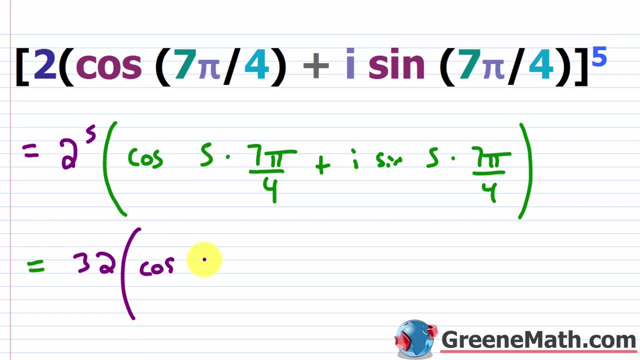 is 35,. so this would be the cosine of: we'll say: let me make that s a little bit better. so we'll say: this is 35 pi over 4, and then we'll say: plus i, so plus i times the sine of 35 pi. 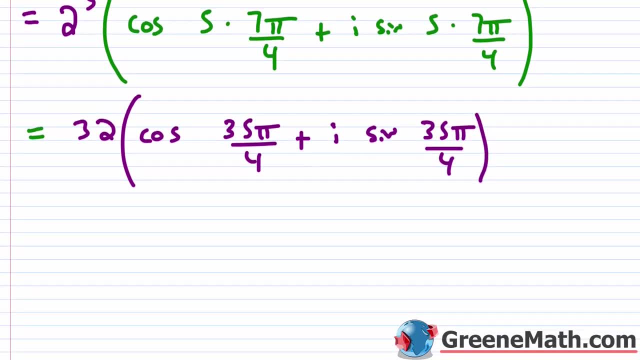 over 4.. Now again, some teachers don't care, You can leave this as your answer. if they say we want it in polar form, It's really up to you If you need to put it in rectangular form. it's kind of hard to do that with 35 pi over 4.. I mean, I know we can use calculators. 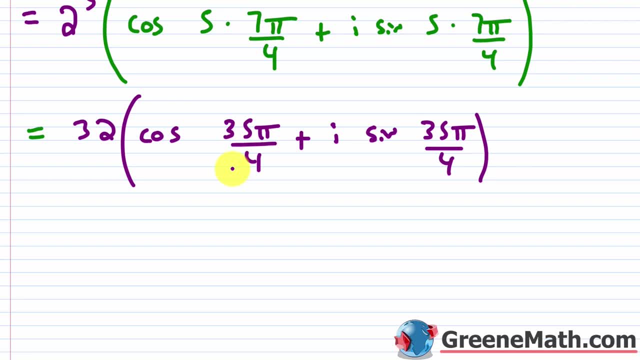 but if you want to do it in rectangular form, you can do it in rectangular form. If you wanted to think about this off the unit circle, for myself, I always like to put it between 0 and 2 pi, with 0 included and 2 pi not okay. So if you think about 35 over 4, forget about the pi. 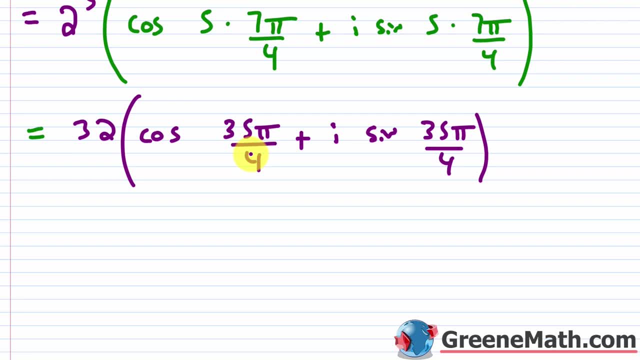 for a second, 35 over 4, that's really close to 36 over 4.. 36 over 4 is not okay. So that tells me, if I think about 2 pi, 4 pi, 6 pi, 8 pi. okay, I would want to subtract 8 pi off to get myself. 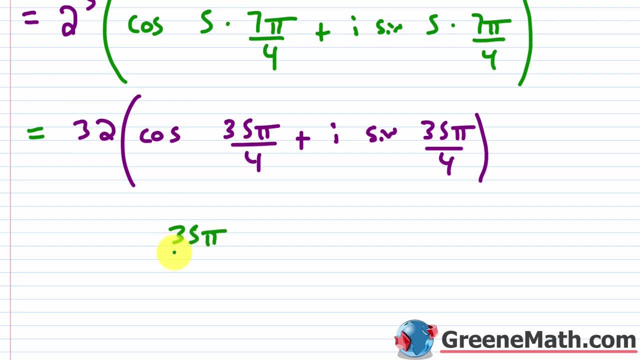 a coterminal angle. So if I did 35 pi over 4, minus 8 pi, of course, I could write that down. this says 32 pi over 4,, 32 pi over 4, this is 3 pi, 3 pi over 4, okay, So it looks a little bit. 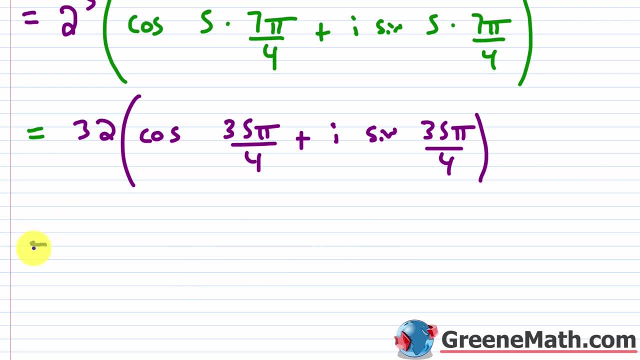 easier to work with. so I'm just going to change this Again. some teachers require it, some don't care. So, 32 times the quantity cosine of 3 pi over 4, let me make that a little bit better, okay. Then plus i times the sine of 3 pi over 4.. Okay, so that's done. So if you want your answer, 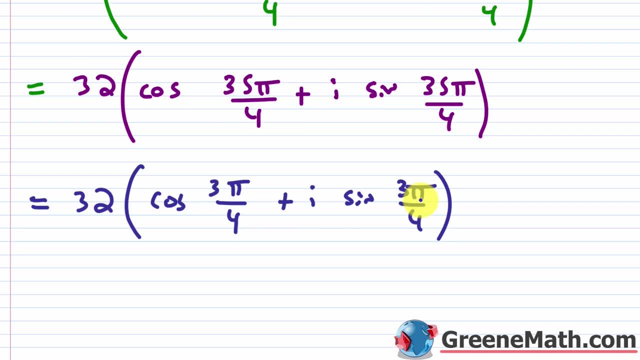 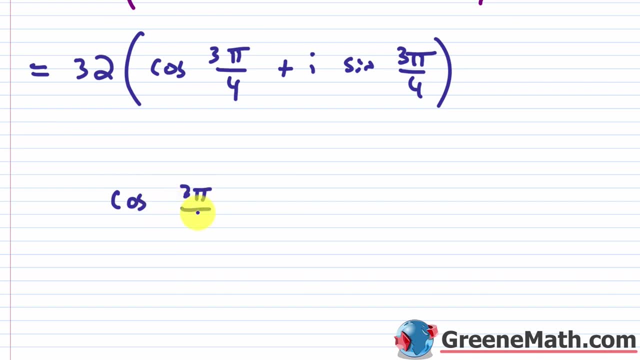 in polar form. again, this one, if your teacher doesn't care, this one, if they do, okay. If you want your answer in rectangular form, well, then again, I've got to go through and figure out, well, what is cosine of 3 pi over 4? And what is sine of 3 pi over 4?? So if you're not, 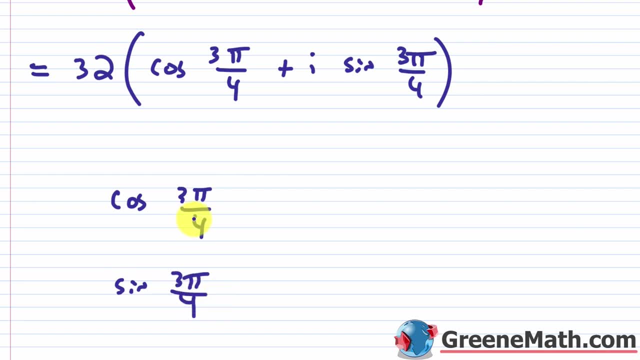 used to working with radians. if you haven't memorize your unit circle, This is 135 degrees, So you know this is in quadrant 2.. So sine is positive, okay, And this guy is negative. And remember, with 135 degrees you have a 45 degree reference angle where, in terms of radians, 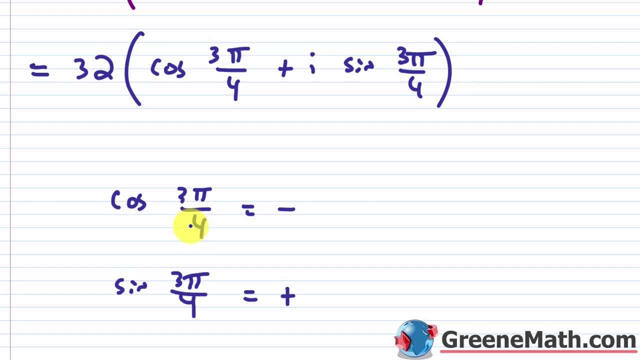 it's pi over 4, okay. So for both of those, it's square root of 2 over 2, if you think about pi over 4, right, But this one's negative and this one's positive. So this would be the negative of the square root of 2 over 2.. And this would be positive. square root of 2. 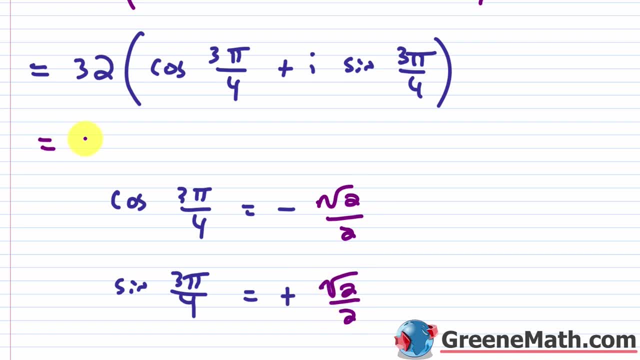 over 2, okay, So we would say that you have equals. I'll go 32 times the quantity. I'd have the negative of the square root of 2 over 2.. And then, plus, you'll have your square root of 2 over. 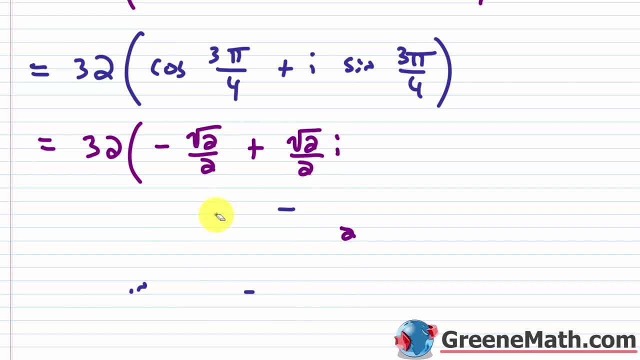 2 times i. okay Again, the i gets changed around based on what book you're looking at, what teacher you're working with. Sometimes they put it out in front there. It's really up to you. So what I'm going to do here is just say that 32 is multiplied by this, 32 divided by 2 is 16.. So this would be. 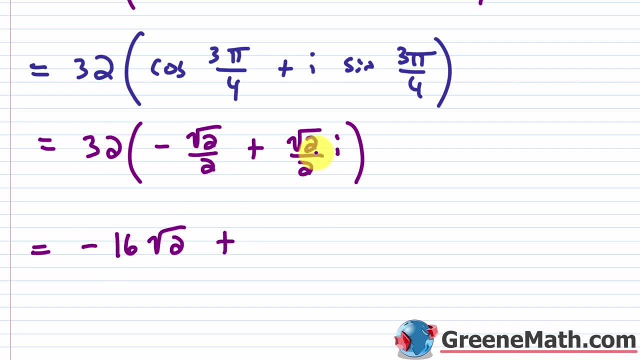 negative: 16 times square root of 2, okay, Plus 32 times this. 32 divided by 2 is 16.. So I'm going to say 16 times square root of 2 and then times i. Now again: this is all over the place in terms of. 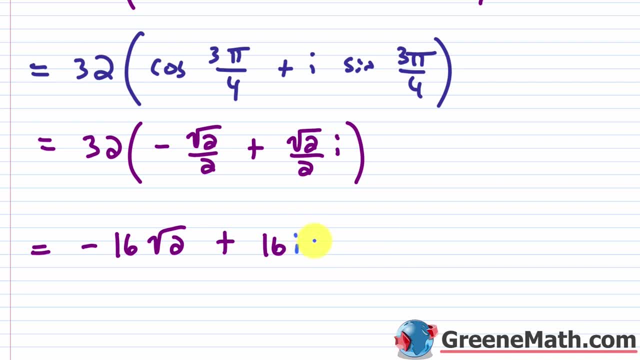 how the formatting goes. Typically with this. you'll see 16i and then times the square root of 2.. Again, you don't want to think that it's underneath this square root symbol, So that's why this is done. okay, So this would be your answer in polar form, right here. 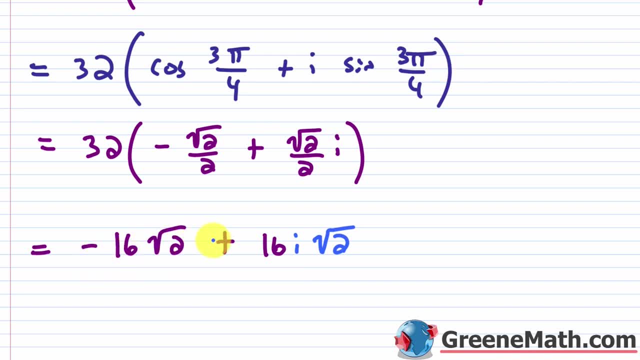 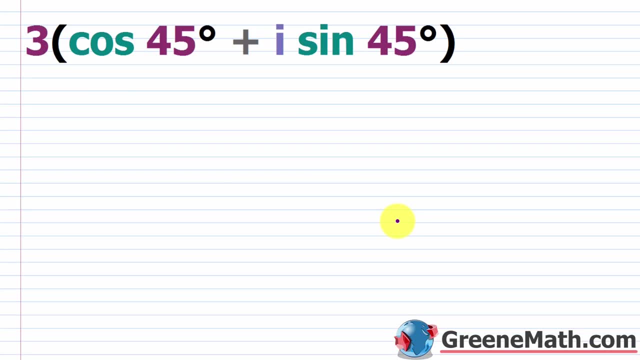 and then in rectangular form, we say negative: 16 times square root of 2 plus 16i times square root of 2.. All right, so now let's talk about the roots of complex numbers. So I'm going to use this first example here to derive a little formula we can use If you don't want to watch it, because 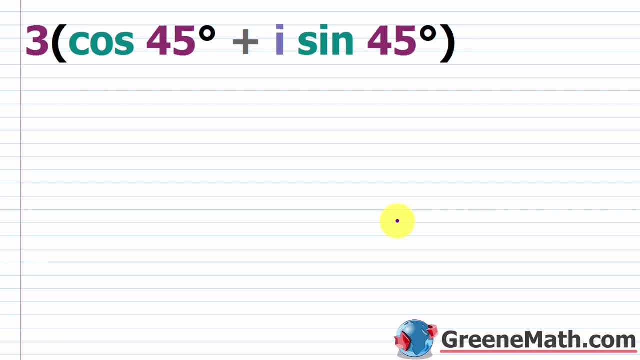 it's a bit tedious, you can just skip ahead to where we're doing the examples. So, first and foremost, every non-zero complex number is going to have exactly n distinct complex nth roots. So you might read this in your book and think: what in the world does that mean? Well, what it. 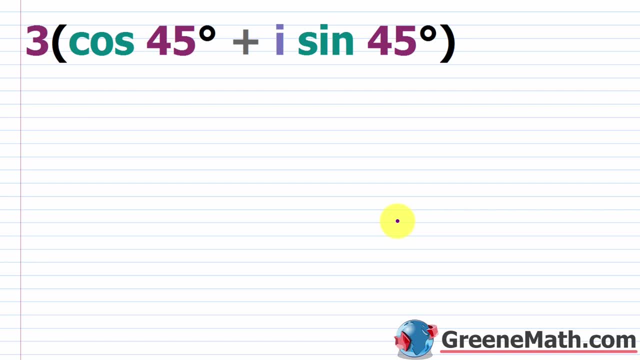 means is that every given non-zero complex number is going to have exactly two square roots, three cube roots, four fourth roots, five fifth roots, so on and so forth. So what we can do is use this example here to come up with a little formula. okay, Let's say that I asked you to find 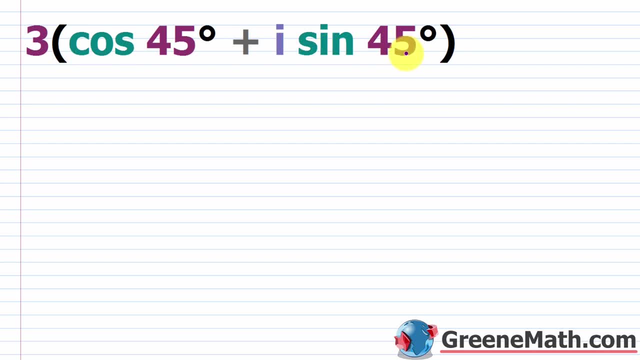 the three complex cube roots of this number. okay, What does that mean? Well, let's just go back to regular numbers. Let's say I had just the number 8, okay, So the number 8.. What if I wanted to? 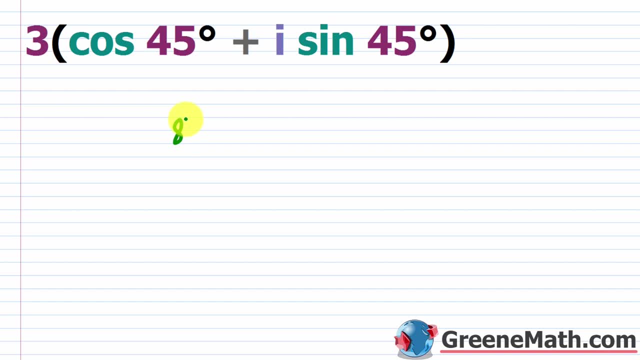 find the cube root of that. Well, I'm looking at the number 8, and I'm going to say, well, I'm looking for a number that, when cubed gives me this number, okay, So we know, this is 2,, right? So 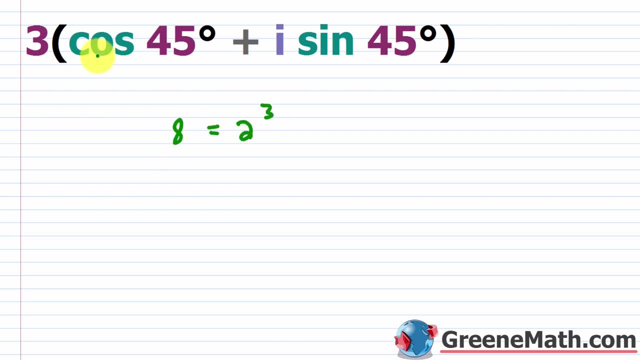 2 cubed gives me 8.. So I'm going to do the same thing. I'm going to be looking for a number that when cubed produces this number here, okay. So all I'm going to do, let me just rewrite this- 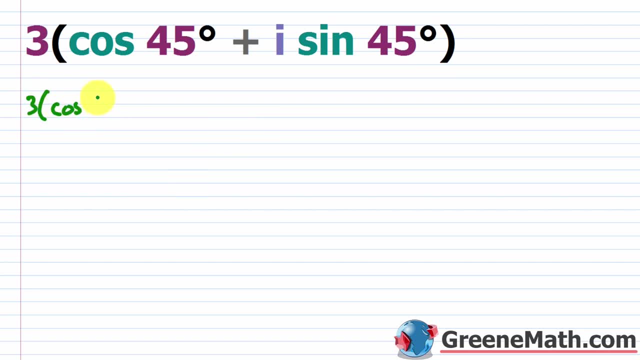 So I'll just say that 3 times the quantity cosine of- let's say 45 degrees, plus the i times the sine of 45 degrees is going to be equal to- again I'm just going to take a generic complex number form. So I'm going to say r times the quantity cosine of. I'm going to use alpha here instead of. 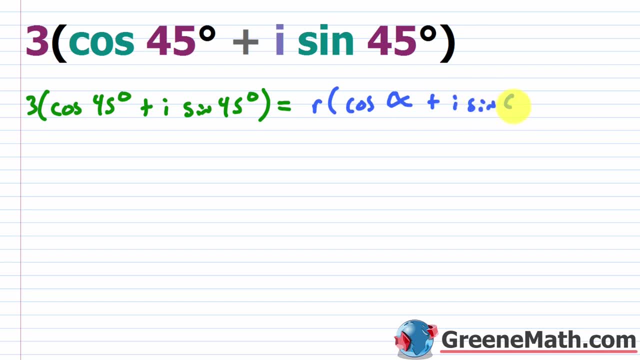 theta. So plus I'll do. i times the sine of again. I'm going to use this alpha, okay, So now I'm just going to raise this to the third power. There is nothing different between this and what I just showed you, with 8 being equal to 2 cubed. okay, I'm just taking this number, raising it to the 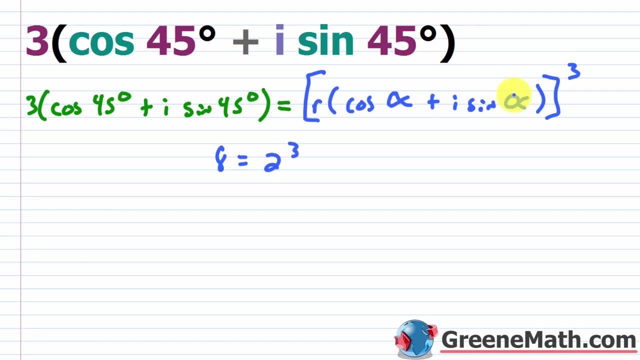 third power. So this number right here is going to be a cube root, okay, of this number, because raising it to the third power produces this, Just like 2 is a cube root of 8, because 2 to the third power is 8, okay, It's all it is. So, from this point on, what I'm going to do is just simplify. 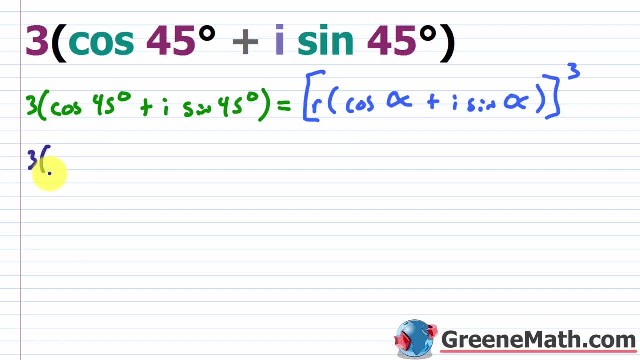 things and come up with a little formula, okay. So I'm just going to say 3 times the quantity cosine of 45 degrees, plus i times sine of 45 degrees. okay, is equal to: if I use my theorem from earlier, r would be cubed, so r cubed and then times the quantity cosine of. I'm multiplying. 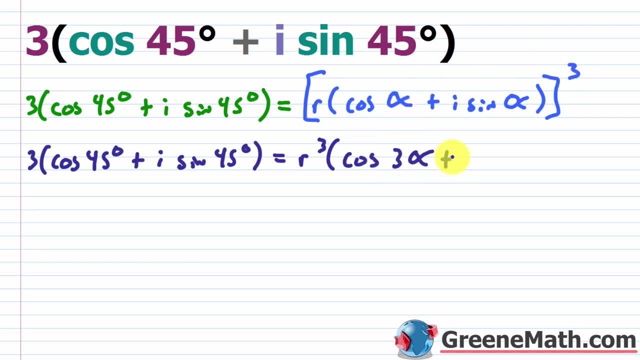 the 3 by the argument, so 3 times my alpha there, plus i times the sine of 45 degrees. So I'm going to multiply this by 3 times the sine of 3 times alpha. okay, So in order for this to be true, 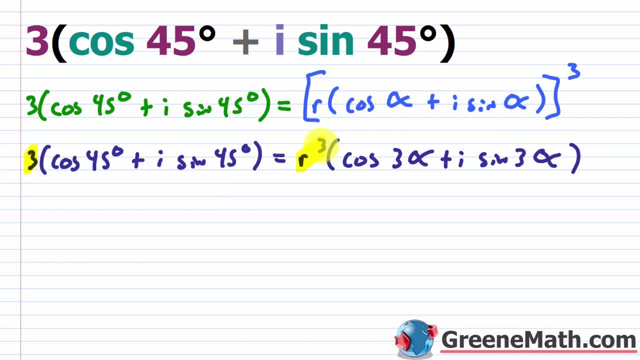 you've got to think about the parts of this equation. So this would have to be equal to this, okay. And then this would have to be equal to this, and then this would have to be equal to this, okay. So in other words, r cubed, r cubed would have to be equal to 3, which tells me, if I take. 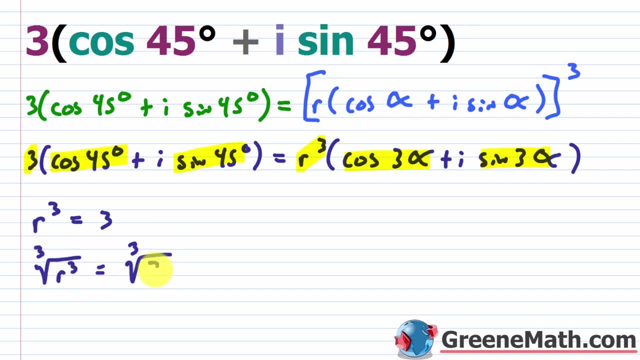 the cube root of each side. okay, the cube root of each side that r is going to be equal to the cube root of 3, okay, And we'll see this in a little bit. So I'm going to take the cube root. 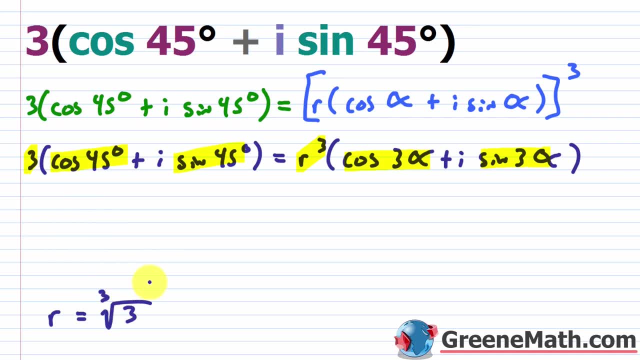 a little formula in a moment, but right now this is what we have, okay, So let me bring this up here, so that it's out of the way, And then the next piece would be that the cosine, the cosine of 45, 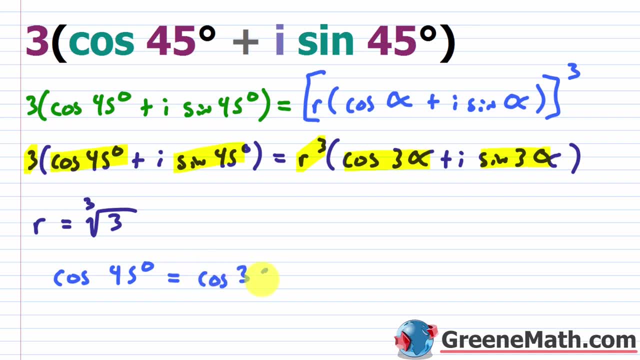 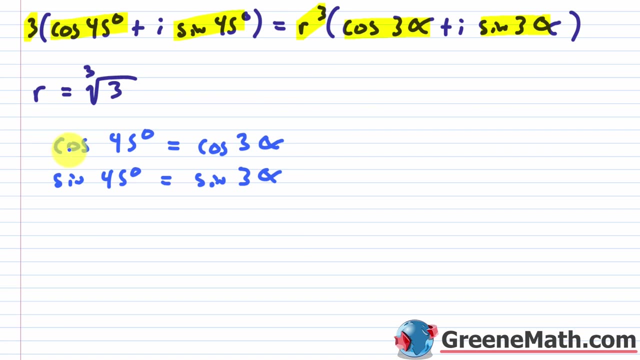 degrees is equal to the cosine of 3 times alpha. okay, And then also the sine: the sine of 45 degrees is equal to the sine of 3 alpha, okay. So let's think about this for a moment. We know about coterminal angles, okay, And we know that let's say, the cosine of 3 times the cosine of 3. 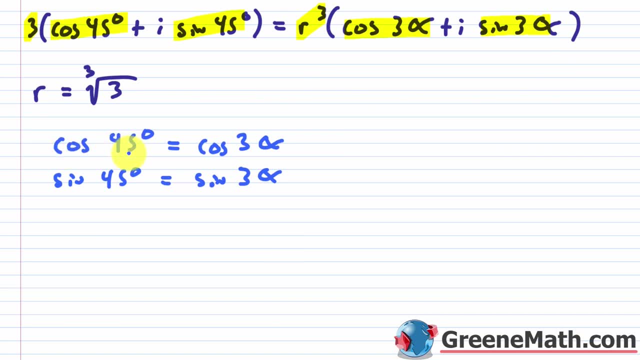 cosine of 45 degrees has the same value as the cosine of if I added 360 degrees to that. So if I said the cosine of 405 degrees, this would be equal to the cosine of 45 degrees, And you can pause the video and punch into your calculator. You should know that those are equal. It's also. 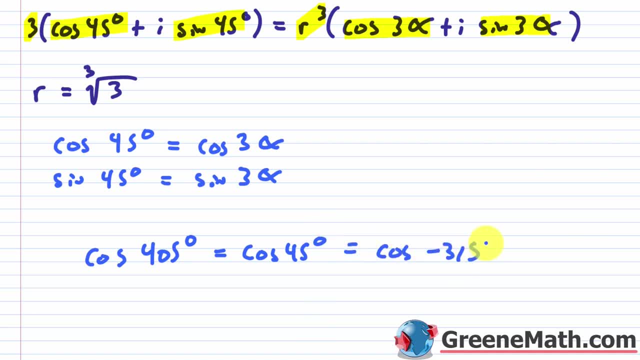 equal to the cosine of a negative 315 degrees. Okay, If you want to do it that way, Okay. So, knowing this fact, what we could do is set three times alpha. So three times alpha equal to this 45 degrees. Okay, Plus I'm going to do 360 degrees times some integer K. Okay, Now we don't have to. 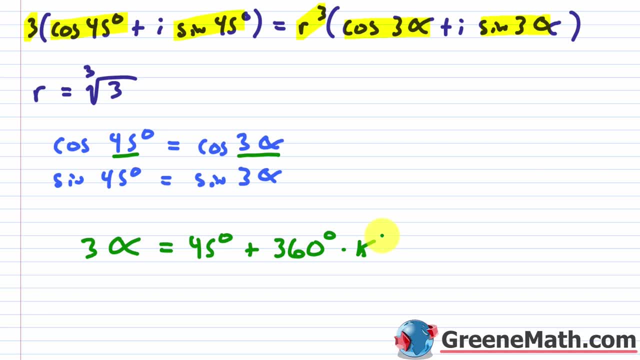 consider negatives. I'm going to show you how solutions just keep repeating themselves. I'm just going to work with zero, one and two Okay, And I'll show you that when you get to three, four, five, six, things repeat Also if you go negative, one negative, two, negative, three. 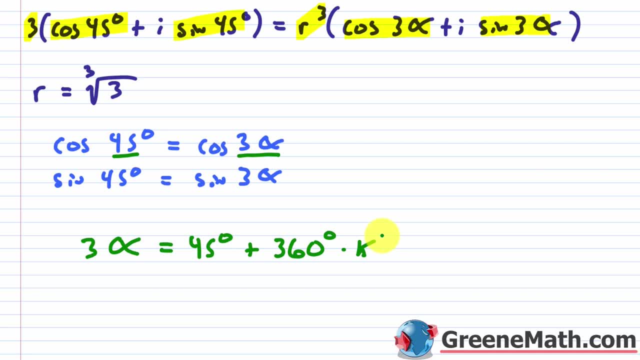 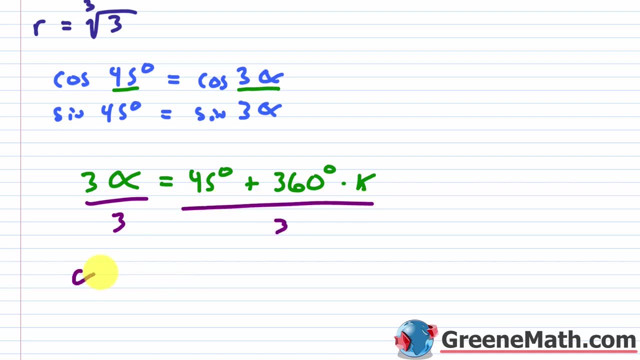 you're just getting repeat solutions. Okay, So what I would do here is I would simplify this a little bit and I would divide both sides by three. Okay, So, both sides by three. So I'd have that alpha is equal to 45 degrees. divided by three is: 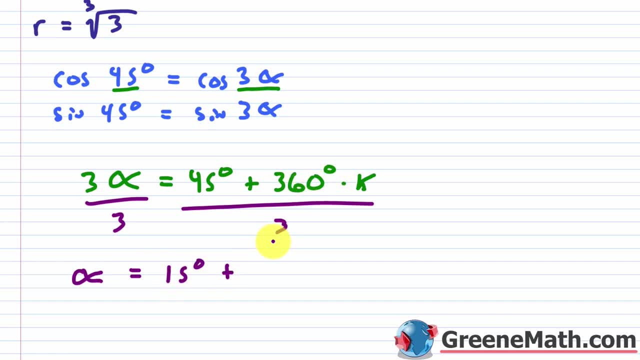 15 degrees, Okay. Then plus 360 degrees, divided by three is 120 degrees, and then times K, Okay. So to get the values for alpha you're going to see in our little formula you plug in: if I'm trying to find the cube root, then I'm going to plug in zero, one and two, Okay So. 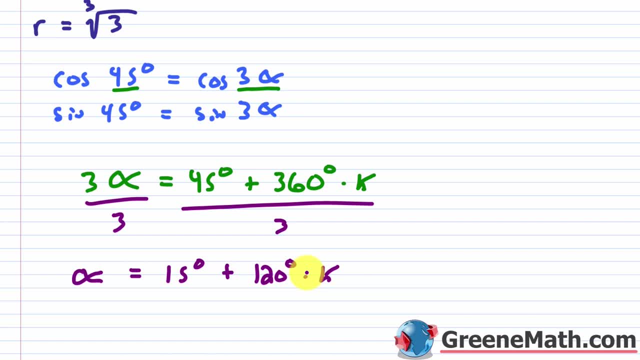 I start with zero, then I go to one, then I go to two. If I was trying to find the fourth root, I would go zero, one, two, three. So it's always one less then that number. Okay. So if it's four, you're going to three, If it's five, you're going to. 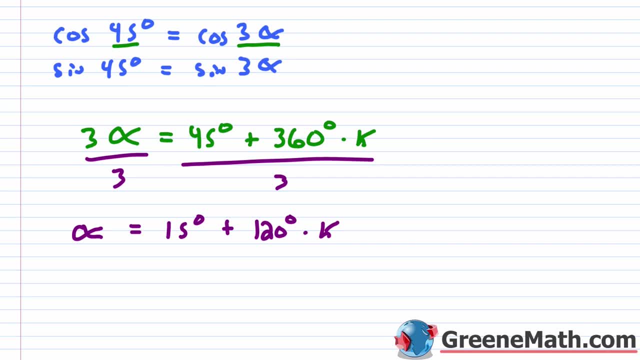 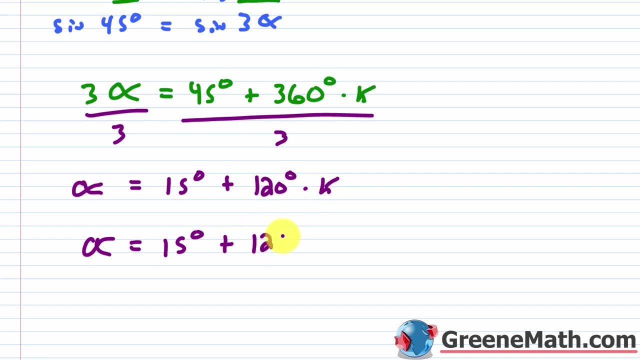 four. If it's six, you're going to five, you know, so on and so forth. So let's go ahead and go through and say our first alpha would be 15 degrees plus 120 degrees times zero. So 120 degrees times zero. So this is basically going to be 15 degrees. Then another alpha would be 15. 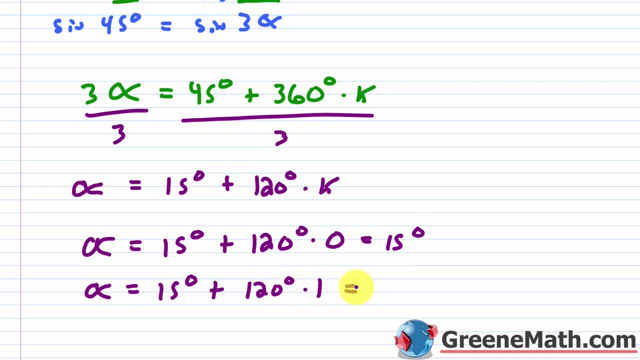 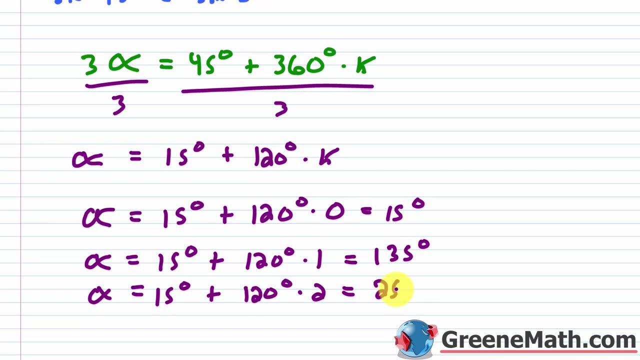 degrees plus 120 degrees times one. So this is going to be 135 degrees. So 135 degrees. then our other alpha is going to be 15 degrees, Plus you're going to do 120 degrees times two And this is going to give me 255 degrees. Okay, And then again we don't need this. 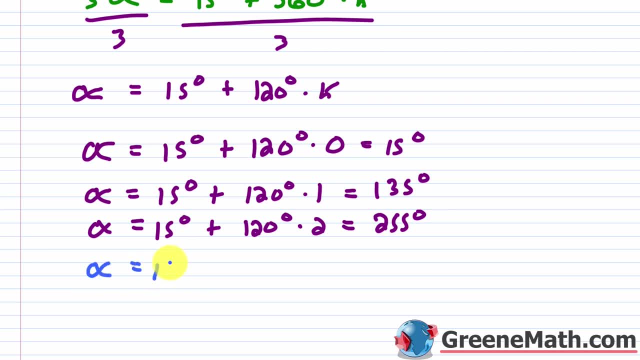 but if you did go to three, so alpha is equal to 15 degrees plus 120 degrees times three. Well, this is 360 degrees plus 15 is 375 degrees. 375 degrees and 15 degrees are co-terminal angles. Okay, So if I was to say the cosine of, 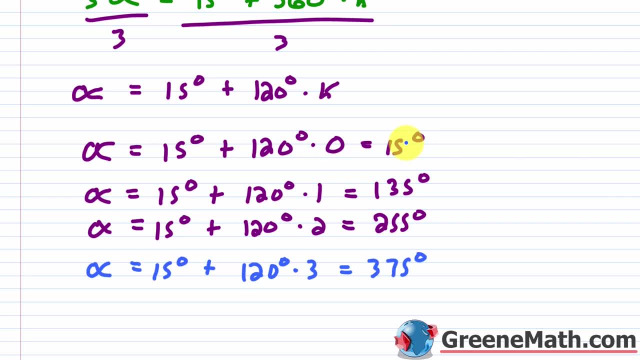 15 degrees or the cosine of 375 degrees, it's the same. Okay, So you don't need to go three and four and five and six. You're just going to get repeat solutions. Okay, So you don't need that. You also. 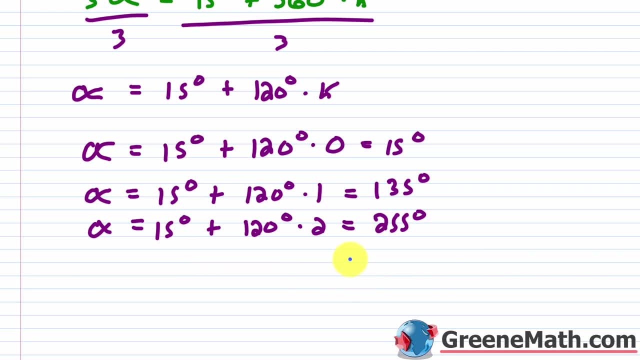 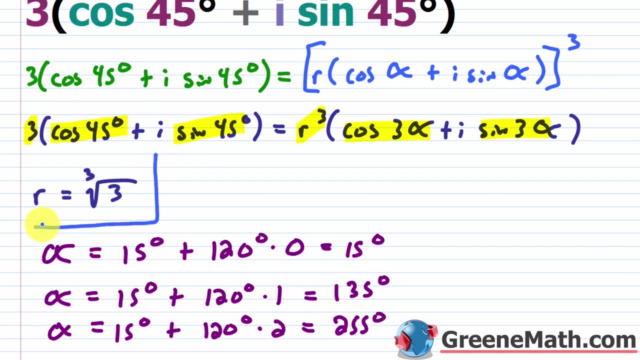 don't need to do the negatives because you're just going to get repeat solutions. So let me erase this. So, coming back now, let me show you that these solutions work. Okay, So let me box this off. Remember, originally we were looking for the three cube roots, So the three numbers that I 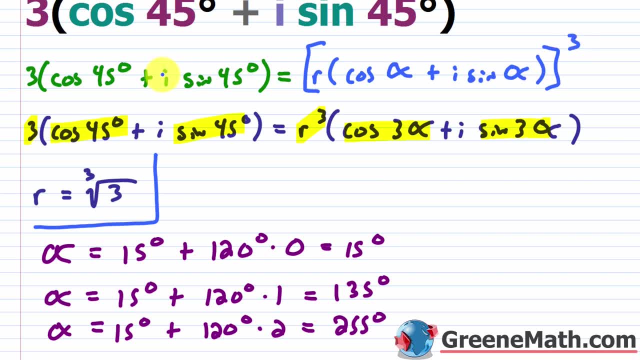 could plug in here and cube them and get back to this number. So let me show you what the first solution for alpha. So we have our R value, which is the cube root, Okay, Of three, And then it's multiplied by the quantity cosine of alpha. So one of those would be 15 degrees plus I times. 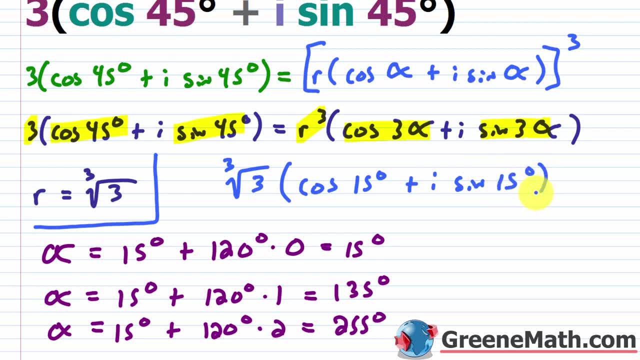 the sine of 15 degrees. Okay, Let me get rid of this one. Then the next one would be the cube root of three times the cosine of it would be 135 degrees plus I times the sine of 135 degrees. Okay, Let's get rid of this one. And then 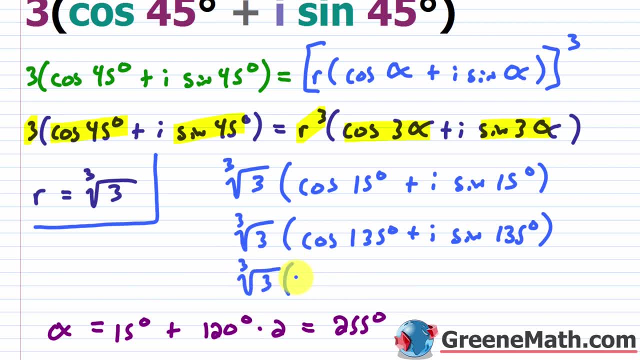 your last root here. So the last cube root would be the cube root of three times the quantity, the cosine of 255 degrees plus I times the sine of 255 degrees. Okay, So let's get rid of this. Now, if you were to cube each one of these, you're going to get back to this right here. 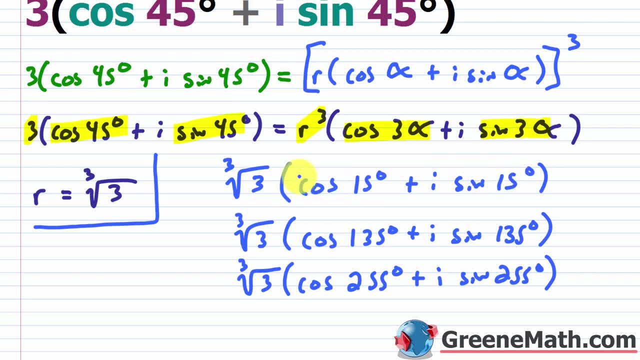 And we can just do it mentally. We don't need to actually go through it. If we cube this number here again, following that theorem from earlier, this guy right here would be cubed. So cubing the cube root of three gives me three, So it gives me back that number. 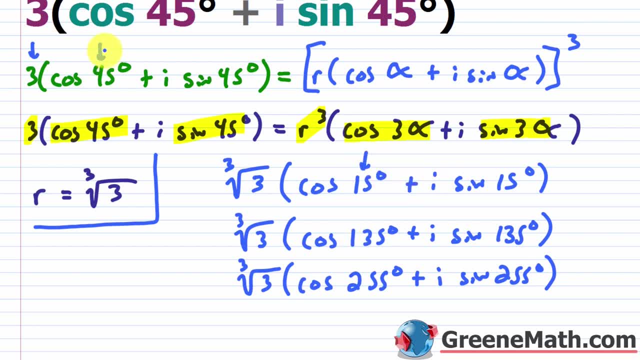 Then if I multiply three times 15 degrees, I get 45 degrees. If I multiply three times 15 degrees, I get 45 degrees. So you can see that cubing this first one right here gives us this back. Now I'll let you do this one and this one on your own. Just cube them. You're going to see. 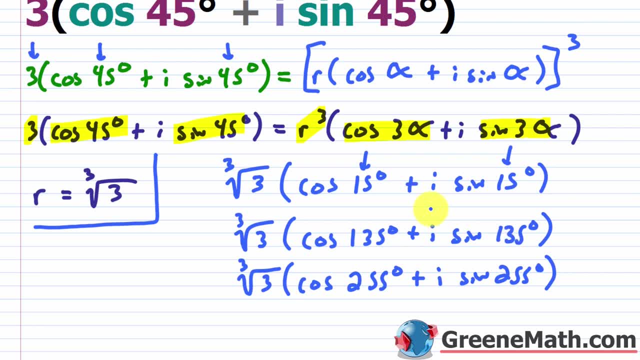 that the angle you get in each case is going to be coterminal with this angle. here, that's 45 degrees, In this case it would be 405 degrees And in this case it would be 765 degrees. Okay, So let's go from our example. 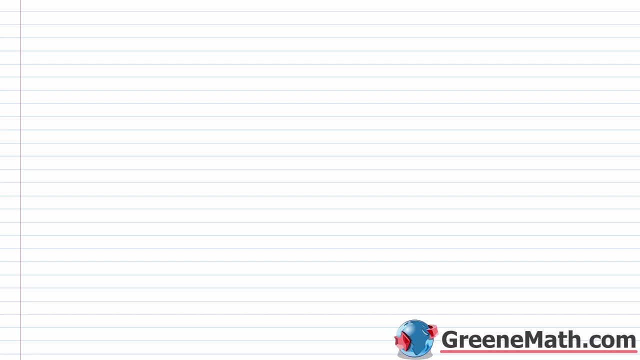 And make a nice little formula. So if n is any positive integer and r is a positive real number and theta is in degrees, then the non-zero complex number, let's say r times the quantity cosine of theta, plus i times the sine of theta, is going to have exactly n distinct nth roots. 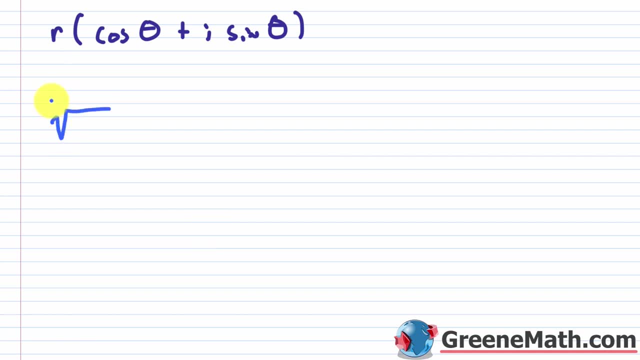 given by the following: So we're going to say that we have the nth root, okay, of this r. You saw earlier we were looking for cube roots, So we had the cube root, which was n. n was three of. in our case it was three, So it was the cube root of. 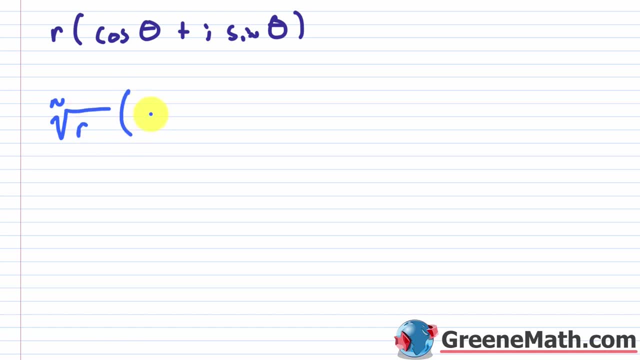 three, Okay, And basically we're going to multiply this by the quantity, You'll have the cosine of alpha, plus i times the sine of alpha. Okay, And basically what alpha is going to be. I'll do degrees first and then I'll do radians, So alpha is going to be theta. Okay, So this guy. 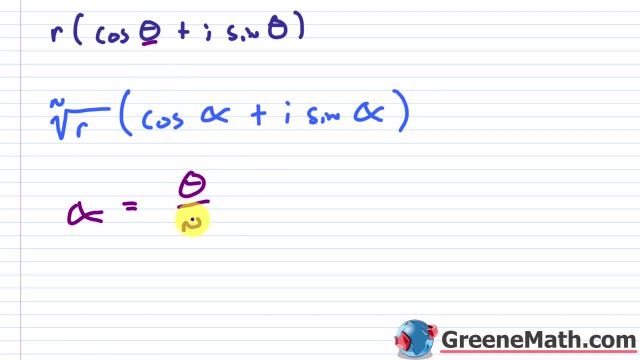 right here, divided by your n- Okay. So you saw earlier, what we had was 45 degrees divided by three, which gave us the cosine of theta, Okay. So we're going to multiply this by the quantity- 15 degrees, Okay. Then plus, you're going to do 360 degrees times k. k is just some integer And 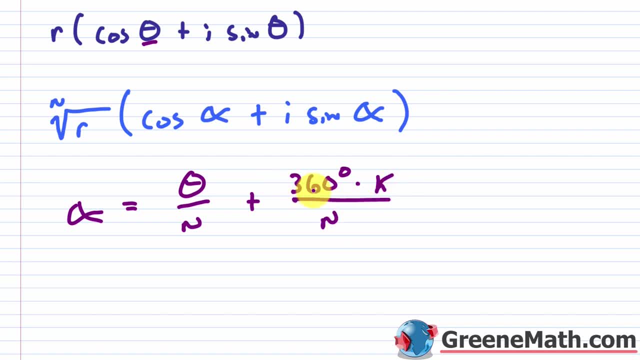 I'll talk more about that in a second. divided by n. So in our example you saw 360 degrees divided by three, Okay, Which gave us 120 degrees, And then multiplied by k, where basically k is going to be equal to zero comma one, comma two comma three. We'll put the three dots here to show. 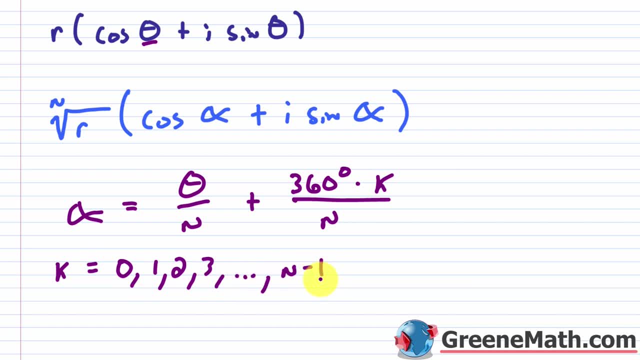 the pattern continues, And then we'll go n minus one, Okay, So in our case our n was three, So we have two, Then three would give us a repeat solution. So with four, so with five, so with six, you know, so on and so forth. Now, if you're working with radians, then you would adjust this. 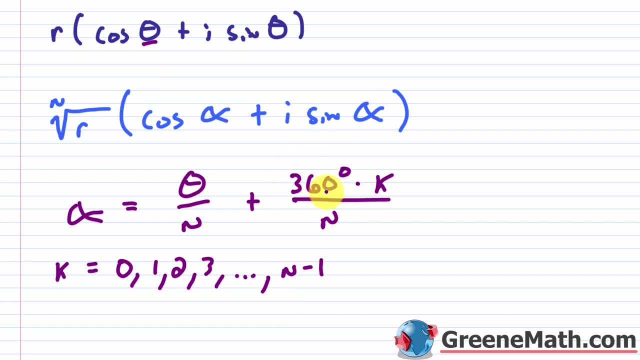 formula And basically, instead of 360 degrees, you would just put two pi in there. Okay, In terms of radians, nothing else is going to change, So just depending on if you're working with degrees or radians. you would either want to use 360 degrees for degrees or two pi for radians. 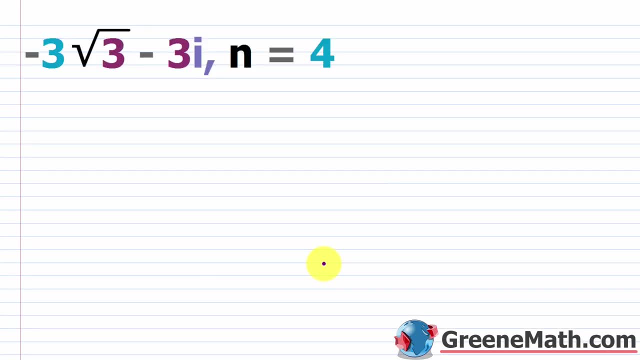 All right, let's go ahead and look at an example. So we want to find all nth roots, Okay, and we're going to write our answer in polar form. So we see that n is set equal to four. So we want to find the four fourth roots, Okay. So I'm going 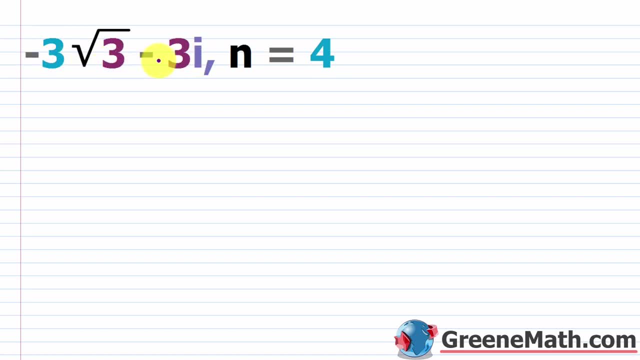 to start by writing this guy right here, this negative three times square root of three minus three i in our polar form. Okay, And so let's go ahead and say that the r value would be what the square root of we take the negative of three times square root of three, we're going to be. 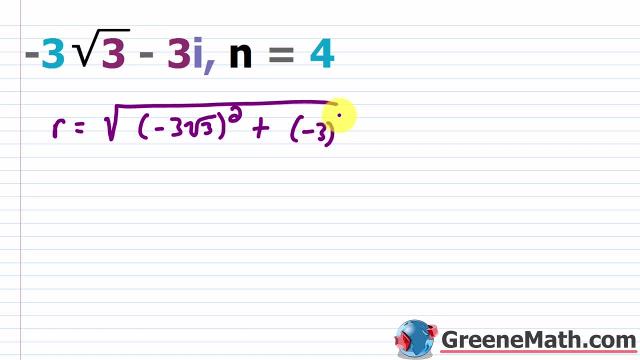 squaring that Plus, you're going to take your negative three. okay, we're going to be squaring that. So the r is going to be equal to. we'll say: the square root of negative three squared is nine. square root of three squared is three. nine times three is 27.. So this is 27 plus negative three. 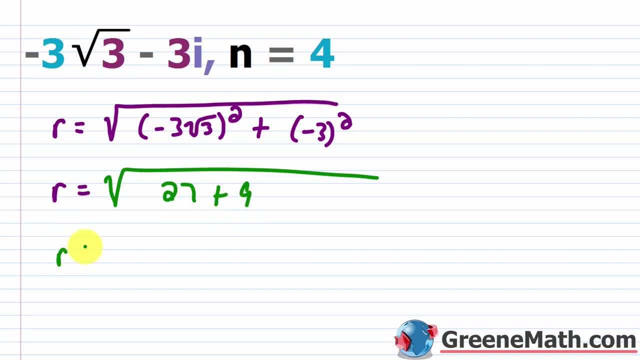 being squared is nine. 27 plus nine is 36.. So r equals the square root of 36.. So r equals six. Okay, so we've got that part down. Let me go ahead and say that, in polar form, this negative. 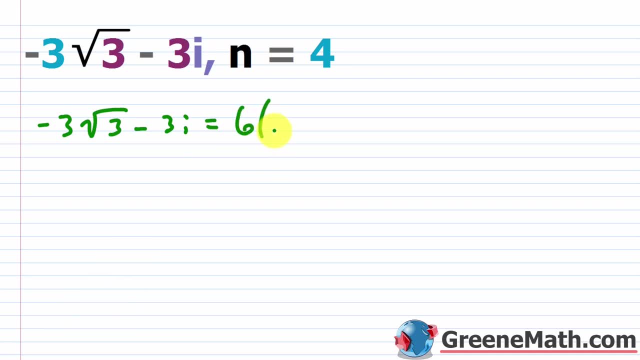 two: I put a six there times you're going to have your cosine, okay, your cosine of theta. I'll replace this in a second, plus your i times your sine of theta, Okay, So for theta again, remember that the tangent of theta is equal to take the imaginary part. so negative three: 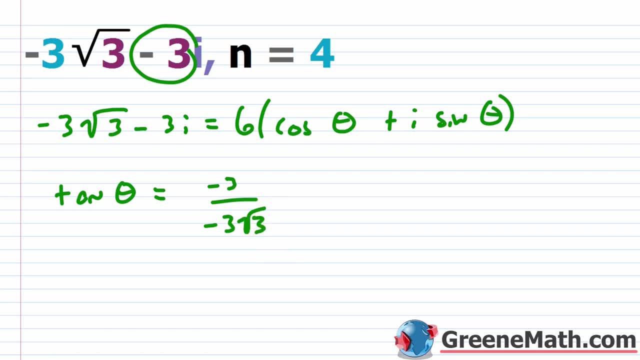 over your real part, which is negative three times square root of three. And so with this we see the negatives are going to cancel, the threes are going to cancel, So you have one over square root of three. again rationalizes the denominator, So square root of three over square. 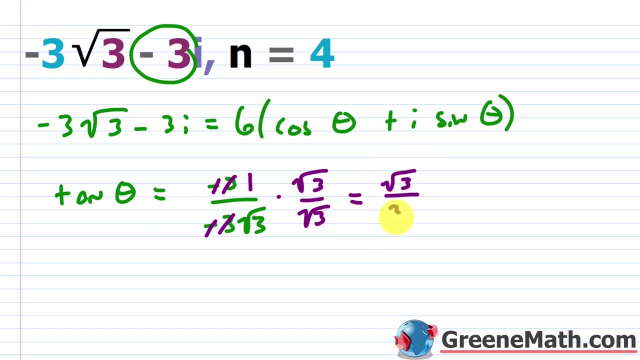 root of three. So this is going to be what Square root of three over three. So if I did my inverse tangent, so my inverse tangent here of square root of three over three, let me make that three a little bit better. If we punch this into our calculator, you're going to get 30 degrees. 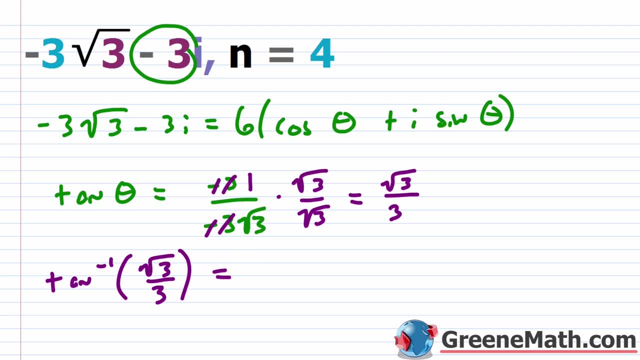 or pi over six. if you want to work with radians, Let's just work with degrees. So I'm going to say this is 30 degrees, So this is my reference angle. So let me erase this And let's think about where this complex number would be if we graphed it. So this is negative and so is this right. So I 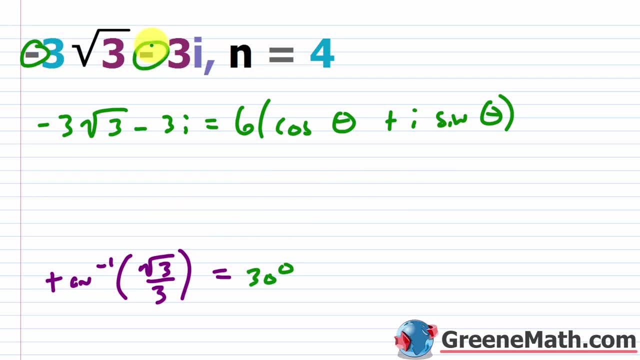 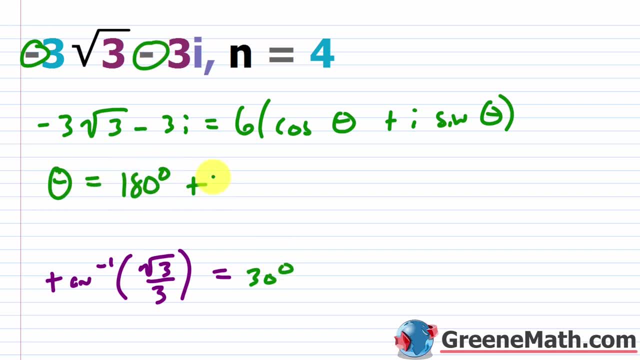 would be 180 degrees plus the reference angle of 30 degrees, which is 210 degrees. okay, So I can just erase this and this and I'll go ahead and put 210 degrees there. So 210 degrees. Once you have this in polar form, it's just a matter of plugging into your formula You want to do. 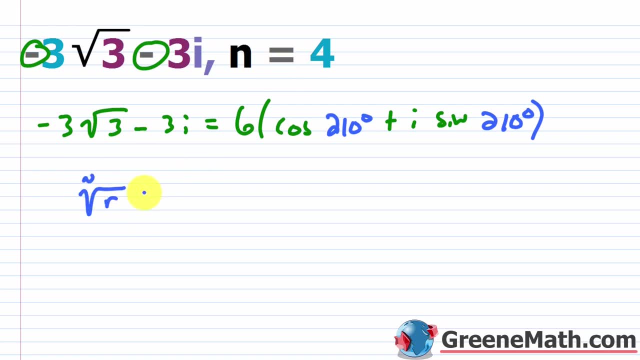 your nth root of r. So in our case, n is 4 and r is 6.. So we want the fourth root of 6.. So we want the fourth root, the fourth root of 6.. And you're going to have four of these, but I'm just going. 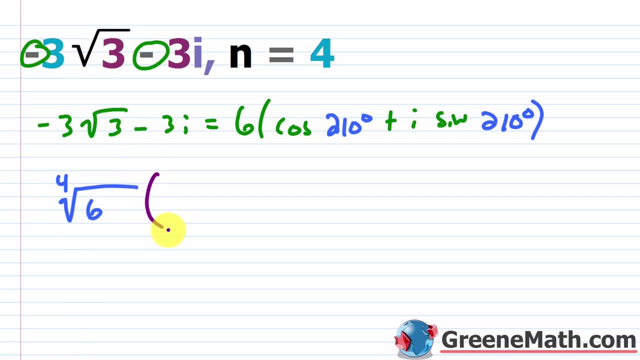 to start out with the first one. okay, Inside of here, what are we going to have? We're going to have the cosine of. again, we call this alpha plus i times the sine of alpha. okay, And alpha, since we're working with degrees, alpha is going to be equal to. you have your theta divided by. 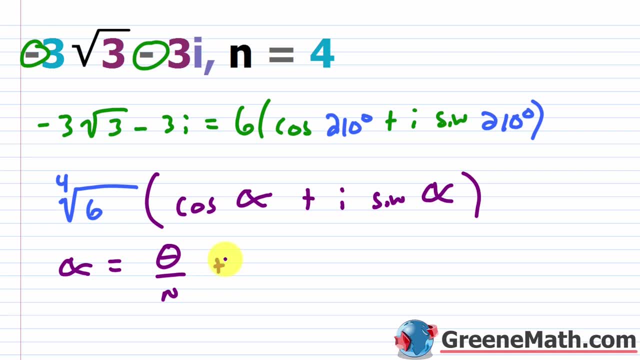 n. In this case the n is 4.. Plug that in a second Plus, you have your 360 degrees divided by n times k, where we say that k is equal to. in this case, because it's 4, it's going to be 0,, 1,, 2,. 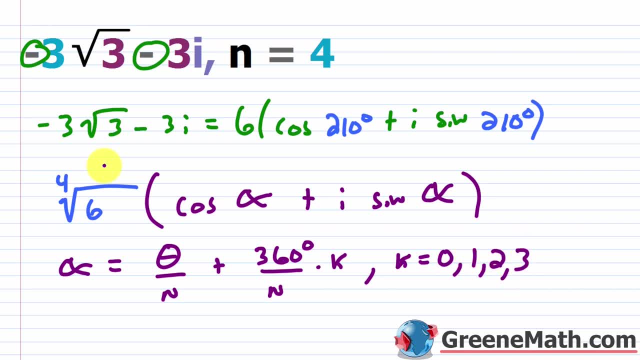 and 3, okay, So you just go up to one less than whatever n is. That's all it is. So in our case, let's just plug this in, So n is going to be 4.. So let's erase this and put 4 in each case. 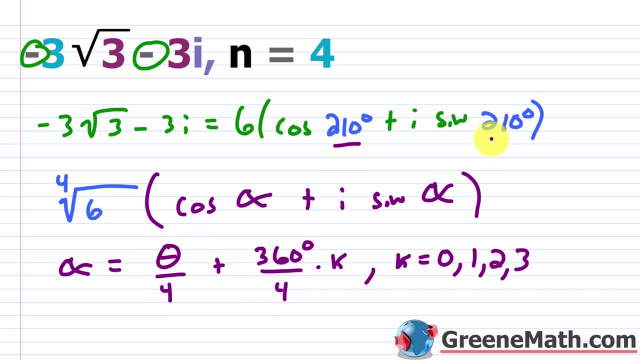 okay. And then theta is coming from here, So it's 210 degrees okay. So let's put 210 degrees here. So if I divide 210 degrees by 4, it's going to give me 52.5 degrees, So 52.5. 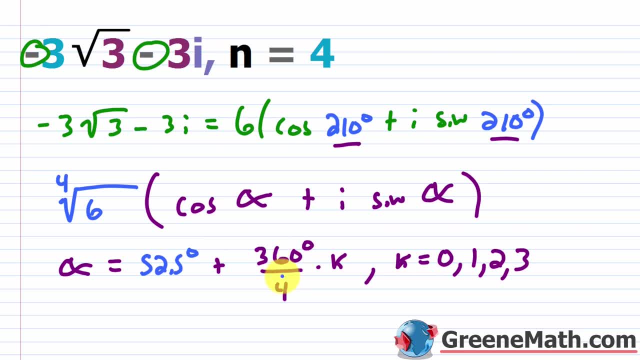 degrees And then 360 degrees divided by 4 is going to give me 90 degrees. okay, So 90 degrees. So basically, to set this up, the first one would be again if this guy was 0, plug that in. 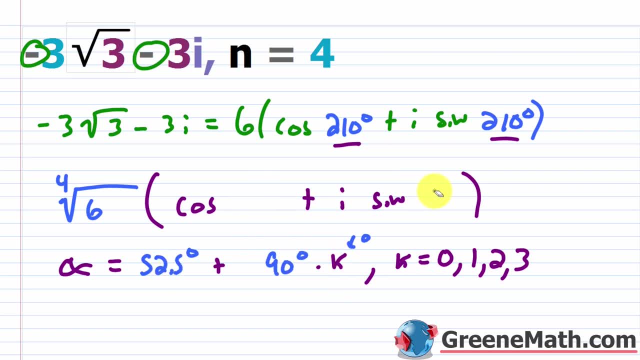 this is gone, So you just get 52.5 degrees. okay, So you can put that in there. So 52.5 and 52.5.. Pause the video and you can raise this to the fourth power and you'll see that you get back to. 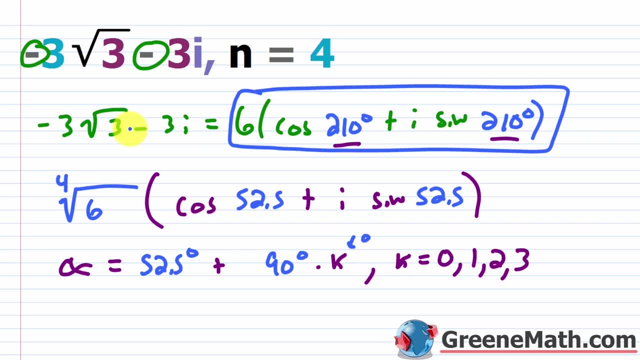 this guy right here, okay, And then, of course, you can convert that back into rectangular form if you wanted to, to get back to that original form we started with. okay, But let's go ahead and keep going And basically, let me drag this down just a little bit and I'm going to slide. 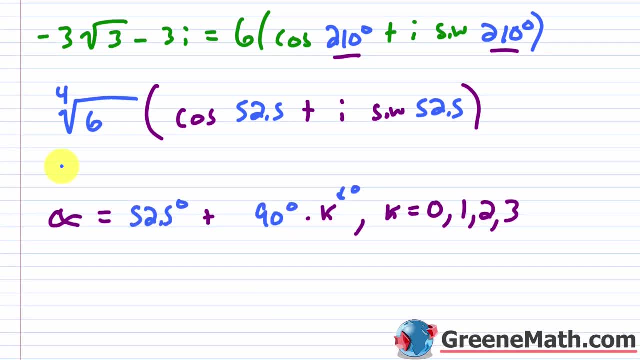 my screen just a little bit down, okay. And basically now I'm going to do the fourth root of 6 times the quantity, I'll do the cosine of and then I'll leave that blank for now, and then I times the sine of. 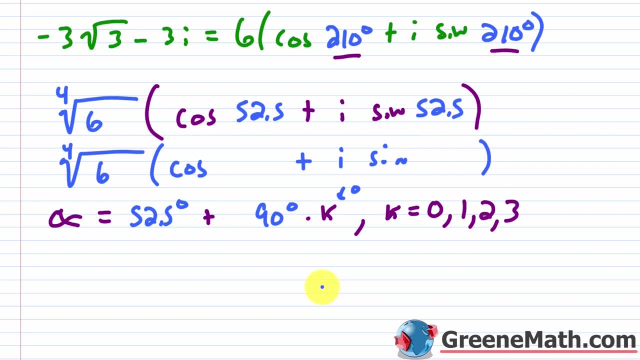 And let me leave that blank for right now. So the next one would be: this guy would be 1 now, okay, So I'm going to plug in a 1.. So basically, 90 degrees times 1 is 90 degrees and 90 degrees. 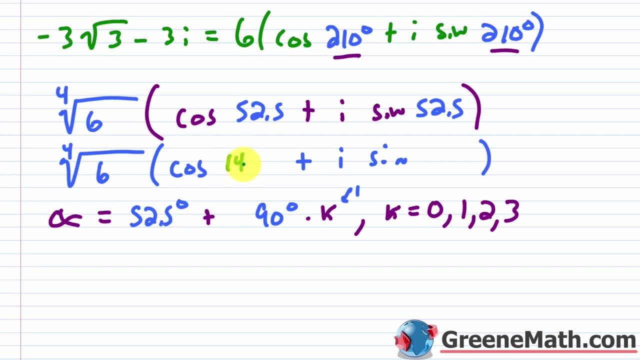 plus 52.5 degrees is going to be 142.5 degrees, And I forgot my degree symbol here and here, so let me put that in. So: 142.5 degrees. let me make that decimal point a little bit better. 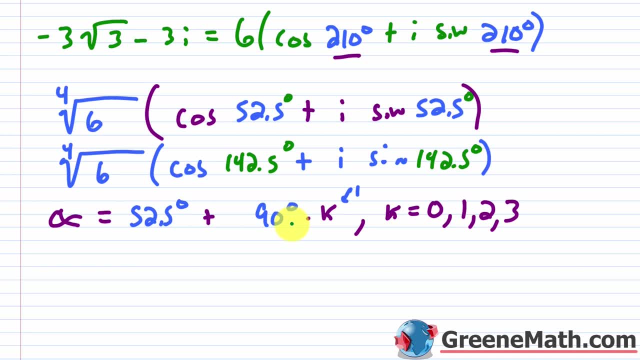 So from here, all I'm going to do is add on 90 degrees, okay, two more times. So I can just get, And basically I can just copy this: And so 142.5 plus 90 is 232.5.. So this would be 232.5 degrees. 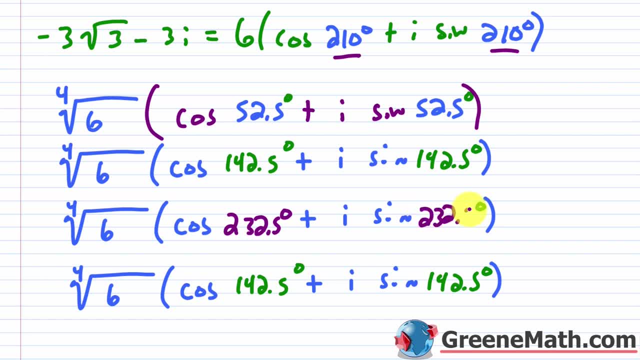 And this would be again 232,, 232.5 degrees, And then add 90 degrees again and you get 322.5.. So 322.5 and 322.5, okay, So this would be your four. fourth roots for that number. I'm leaving. 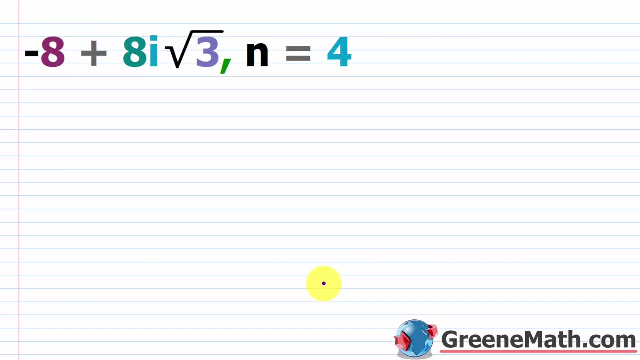 these in polar. All right, let's take a look at another example. I think this is going to be pretty easy for us at this point, But I want to throw something in here. Sometimes your book will ask you to graph the roots on the Argan diagram or the complex plane, So let's go ahead and do this. So we have negative. 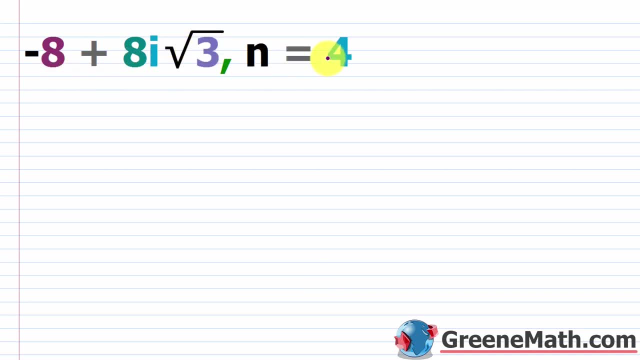 eight plus eight. i times square root of three. Again n is going to be four. So I'm looking for the four fourth roots Now. again, this is given to us in rectangular form, So I need to convert it into polar form first. okay, So the r value times again the quantity cosine of theta. 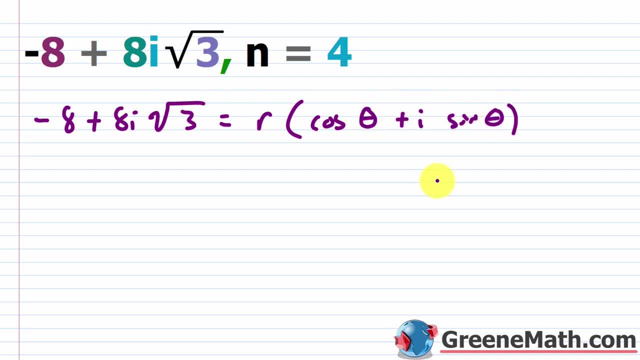 plus i times the sine of theta, So let's do this quickly. So r is going to be what? The square root of negative eight squared is 64.. And then, if you have eight times square root of three being squared, it's 64 times three, which is 192.. Okay, so you're adding those two together. 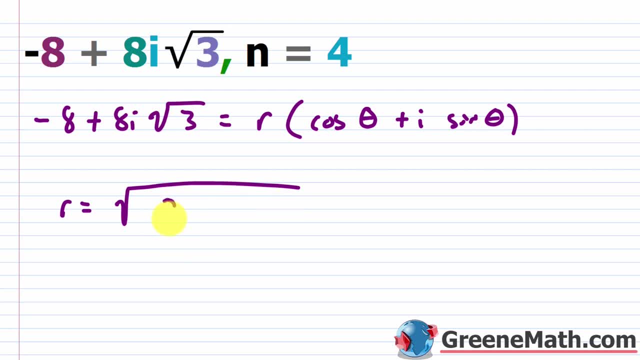 And that's going to give me 256.. If I took the square root of that, I would get 16.. Okay, so let's just erase this and put 16 here. Then for theta, it's going to be where The real part. is negative. So I'm going to put 16 here And then for theta, it's going to be where The real part is negative. So I'm going to put 16 here And then for theta, it's going to be where The real part is. 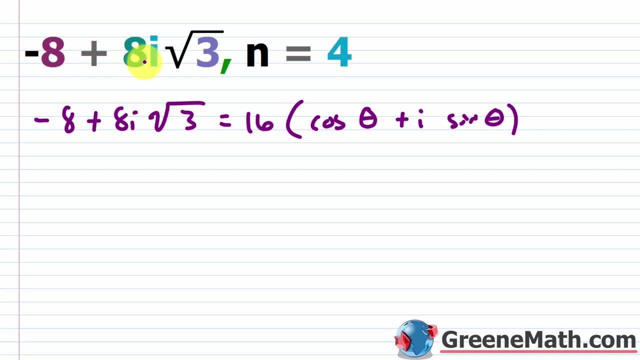 going to the left. The imaginary part is positive. So then I'm going up. So, from the origin, if I go to the left and I go up, I'm going to be in quadrant two. Okay, so let's say that theta will. 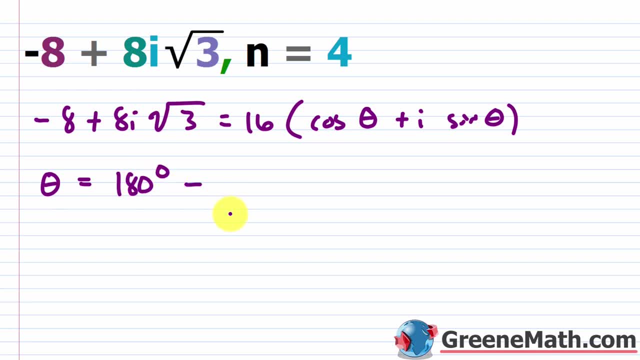 be equal to 180 degrees minus my reference angle And the reference angle here. let's go eight times square root of three And I'm going to divide that by. forget about the negative, let's just do eight. This is going to cancel with this. So this is square root of three. Okay, so I'm going to say: 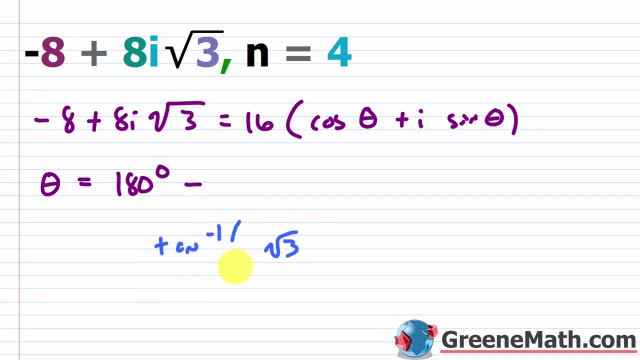 the tangent inverse. the tangent inverse of this guy right here is going to give me 60 degrees, Okay. so if I subtract 60 degrees away from 180 degrees- okay, because this is my reference angle in quadrant two- well, it's going to be 120 degrees Okay. so that's my theta. Let's get rid of this. 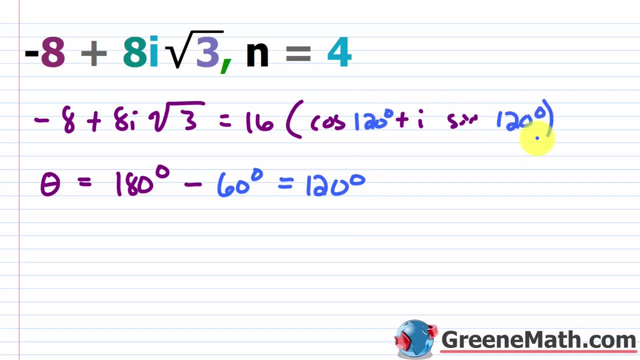 Let's put in 120 degrees and 120 degrees. Okay, so that's pretty quick, All right. so from here I need to get the four fourth roots. So in each case, I'm going to take the fourth root of 16,. 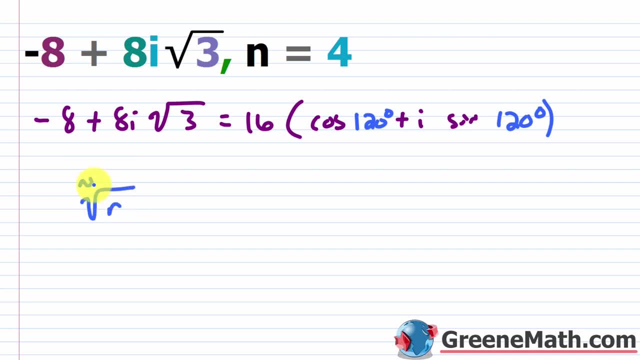 right, Because again, it's the nth root of r, So n is four, r is 16.. So the fourth root of 16 is two. right, Because two to the fourth power is 16.. So I'm going to put two, two, two and two, Okay. 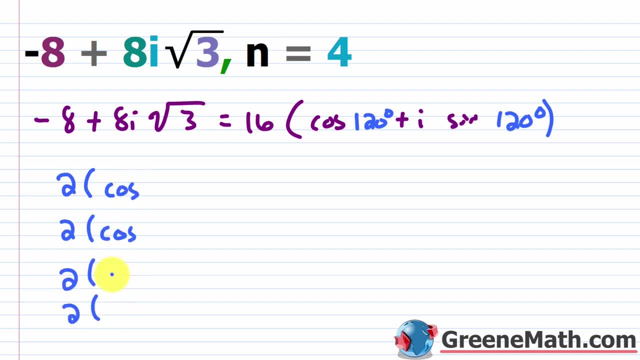 let's go ahead and set this up in each way. So cosine, cosine, cosine and then cosine. Okay, so what's going to go here, here, here and here? Remember, when you think about the formula: if you call this alpha, it's equal to. again, you take theta, okay, which in this case is 120 degrees. 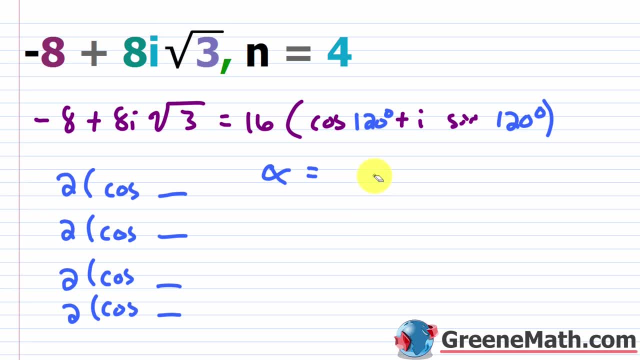 and you divide it by n, So you divide it by four. So in this case that would be 30 degrees. Okay. then plus, you have your 360 degrees times your integer k divided by your n. So 360 degrees divided by- in this case it would be four, would be 90 degrees. Okay, so this would be 90 degrees. 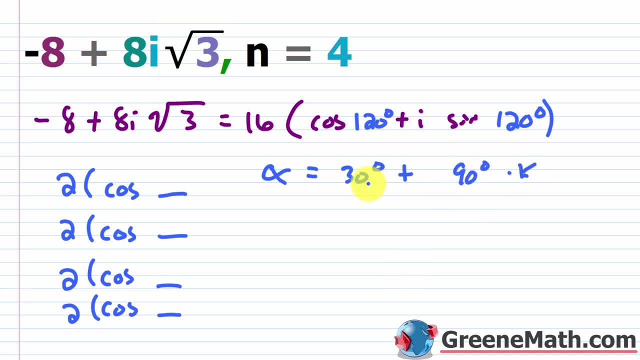 times k. So for the first instance, this would be 30 degrees. So let's go ahead and put 30 degrees here. I'll fill out the rest in a moment. Okay, And the next instance? I'm going to put 30 degrees. 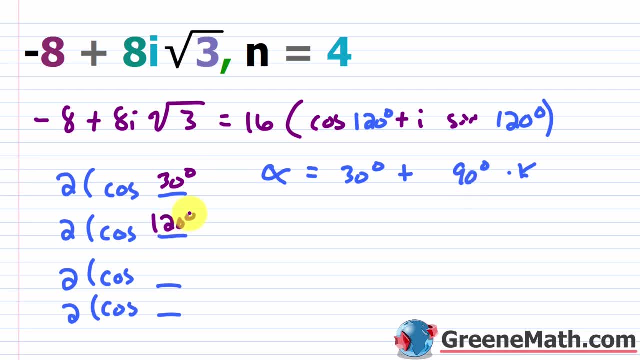 here. So in this instance it's going to be plus 90 degrees, So this would be 120 degrees, then plus 90 degrees, So this would be 210 degrees, then plus 90 degrees, So this would be 300. 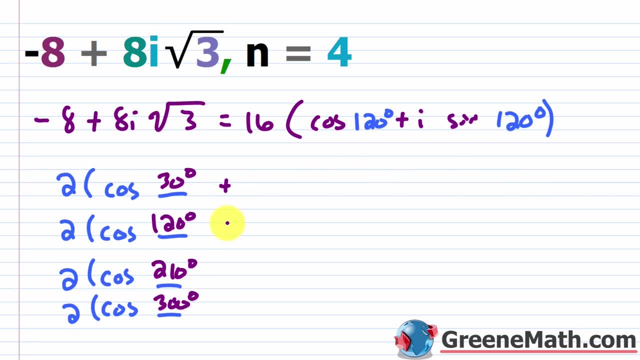 degrees. So let's get rid of this And let's put our plus, plus, plus, plus, i, i, i and i, and then the sine, the sine, the sine and then the sine of 30 degrees. close that down And this. 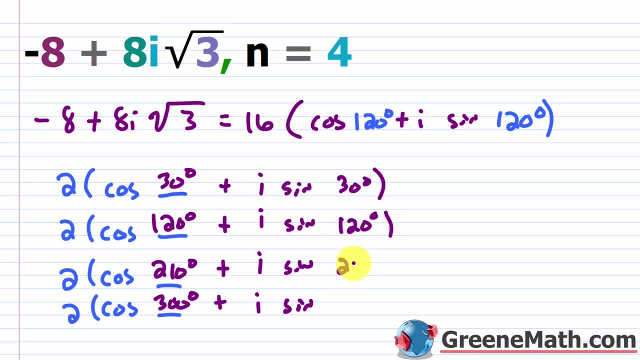 will be 120 degrees- close that down- and then 30 degrees. So this would be 120 degrees and then 210 degrees- close that down- and 300 degrees. Okay, So these are our four fourth roots, okay. 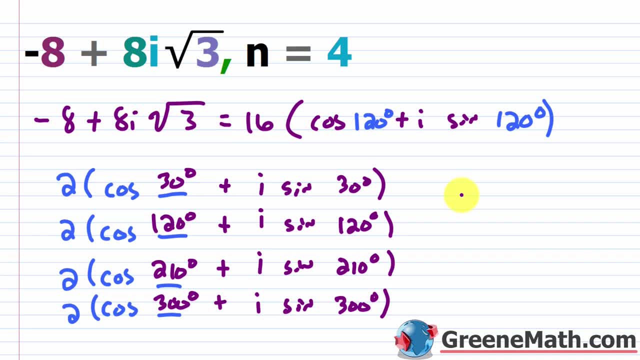 for this number in polar form. Okay. so how would we go about graphing these complex roots? Well, basically, each of these can be represented as a position vector in the complex plane. So notice that your magnitude in each case is two. Okay, so two, two, two and two, So what you could. 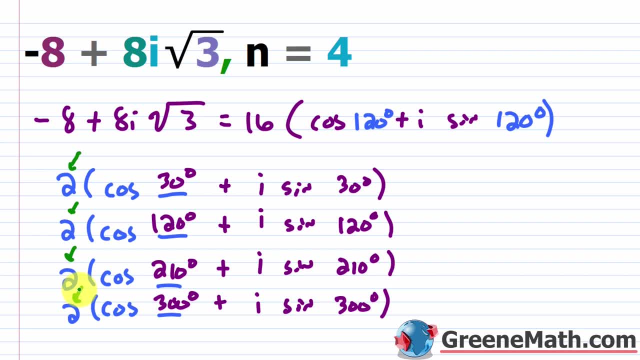 do to represent. that is, you could have a little circle with the center, at the origin and where the radius is two. Okay, So each one of these can be represented as a position vector in the complex plane. Okay, So notice that your magnitude in each case is two. Okay, so two, two, two and two. So what? 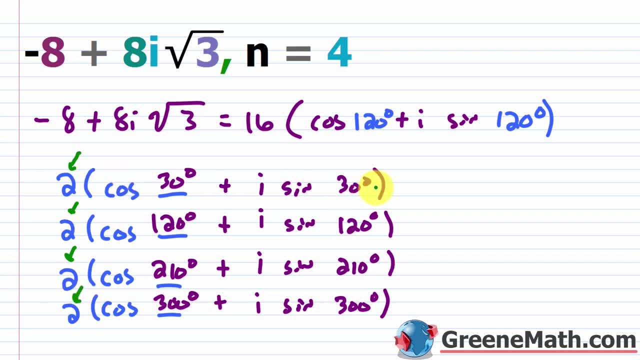 these as a vector is going to have an initial point at the origin and the terminal point that's going to touch that circle that you drew, Okay, And then, in terms of the direction angle for the vector, just get it from here. So the first one will be 30 degrees, the second will be 120 degrees. 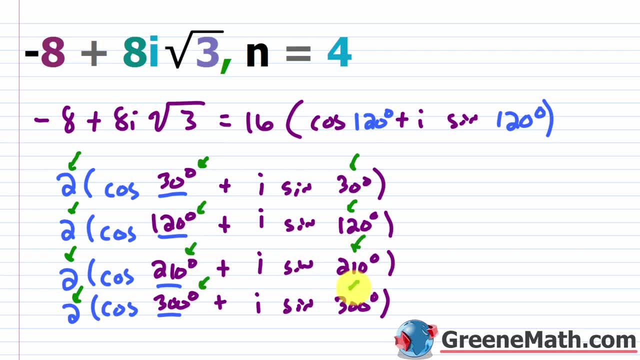 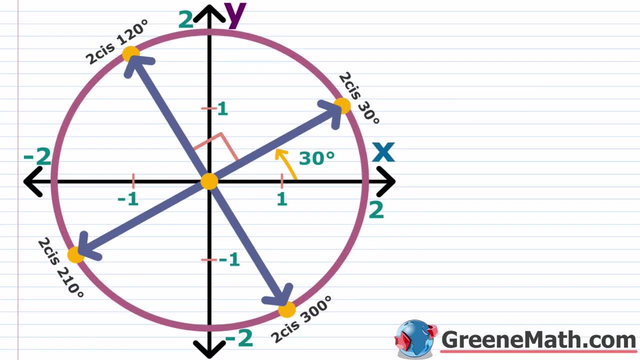 the third will be 210 degrees and the fourth will be 300 degrees. Okay, So these guys are going to be spaced 90 degrees apart. Okay so, equally spaced 90 degrees apart. So if we go to our little coordinate plane- and I know that most people put imaginary here, so you can put that- 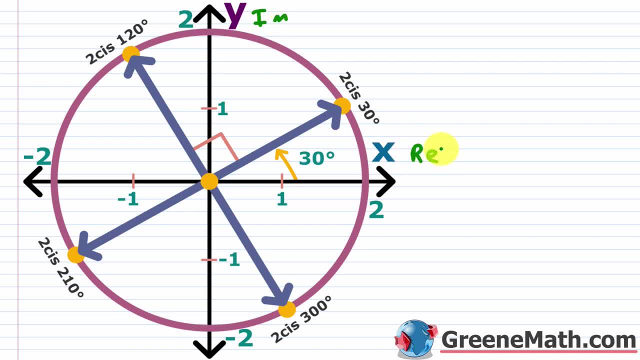 if you want. So you can put imaginary And then for this you could put real. But again, if you write this as x plus y, i, then x could still be your real axis and y could be your imaginary axis. It's really up to you, or your teacher, Okay, so I'm just putting it this way. So when we think, 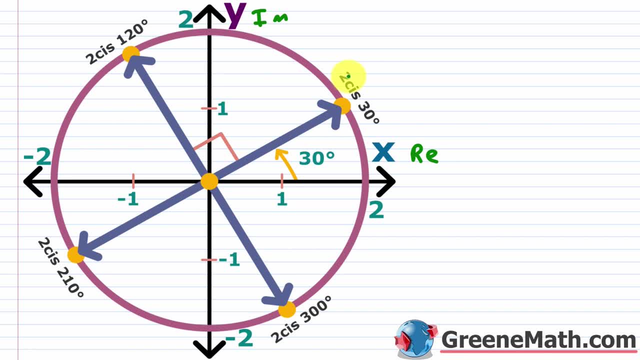 about this again. the first solution was two times the quantity of the cosine of 30 degrees, plus i times the sine of 30 degrees. we abbreviated it here, But you can see that I have a position vector. the initial point is at the origin. the terminal point is going to touch this little. 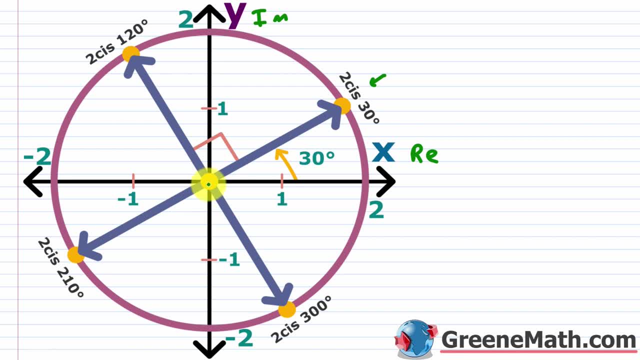 circle that I drew, okay, with a radius of two and a center at the origin, Okay. so you see that this is a 30 degree angle, Okay, And then if we go another 90 degrees here, so this is another 90. 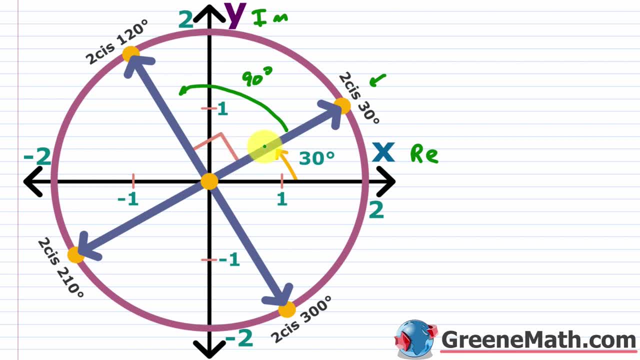 degrees. you can see that little 90 degree symbol there. Basically I'm going to get to my next solution. So the angle here is 120 degrees. Again, if I started here, 30 degrees plus 90 degrees gives me 120 degrees- okay for the whole thing. And then basically you can see that it touches. 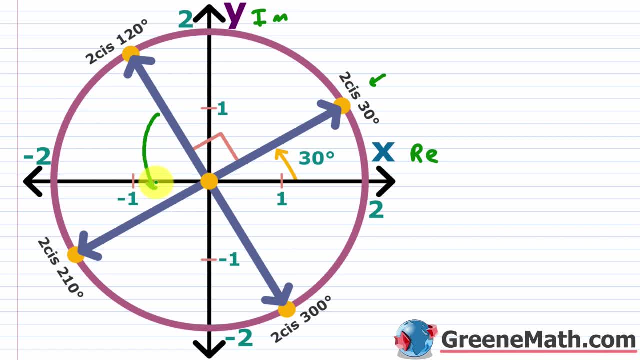 again our little circle. If we keep going around, this is another 90 degrees, and then this is another 90 degrees. Okay, so it keeps putting you to another solution. So this angle here: if I started here and went all the way to here, this is 210 degrees If I started. 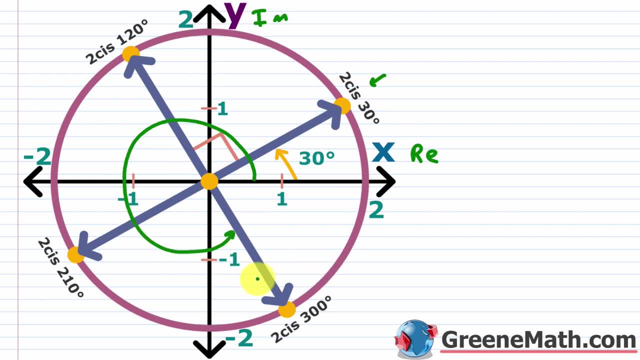 here and went all the way around to here. this is going to be 300 degrees. Okay, so that's basically how you can sketch the graph If you're given this as an assignment. again, just take your magnitude- okay, in each case, ours was two- and draw yourself a little circle with the center of the 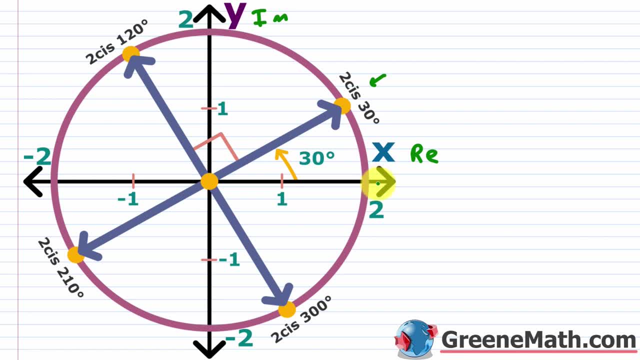 origin and the radius of that number. Okay, in our case it's two. Then what you want to do is have position vectors So they start at the origin and their terminal point is going to be on that circle And your direction angle in each case is given by the angle. So here it's 30 degrees. 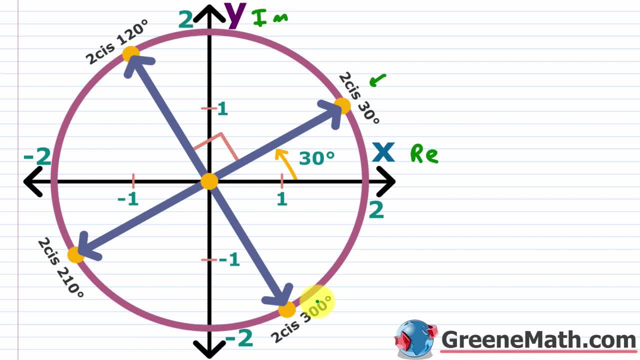 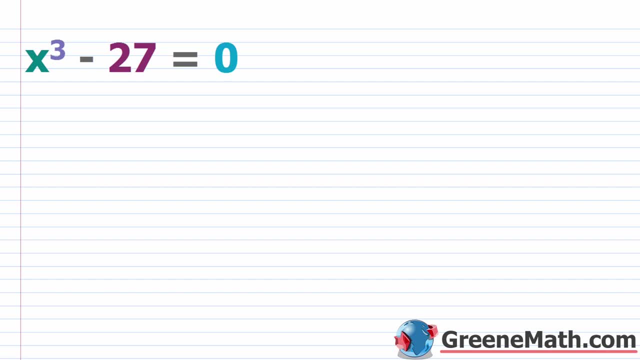 here it's 120 degrees, here it's 210 degrees and here it's 300 degrees. All right, so let's wrap up the lesson and look at another example. Here we're going to be solving a simple equation using the roots of a complex number. Okay, let's say we saw something like x cubed minus 27. And this was: 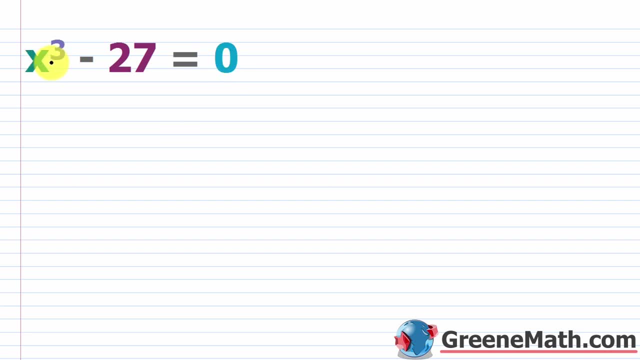 equal to zero. The first thing we know that, since this is a complex number, we're going to be able to solve a simple equation using the roots of a complex number. Okay, let's say we saw something like x cubed minus 27. And this was equal to zero. The first thing we know that, since this 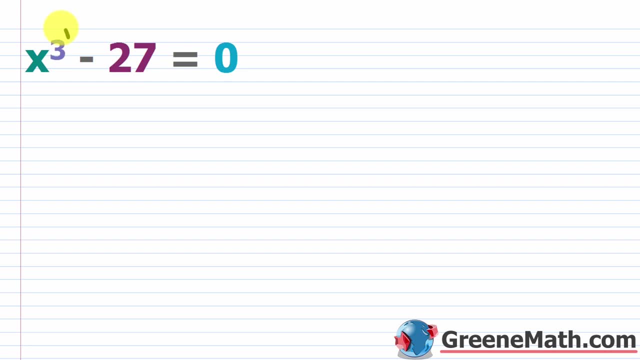 polynomial here is of degree three. okay, we have this exponent of three here and not higher. Well, we know we're going to have exactly three complex solutions for this equation. Okay, that's the fundamental theorem of algebra. So how could we use the roots of a complex number to solve an? 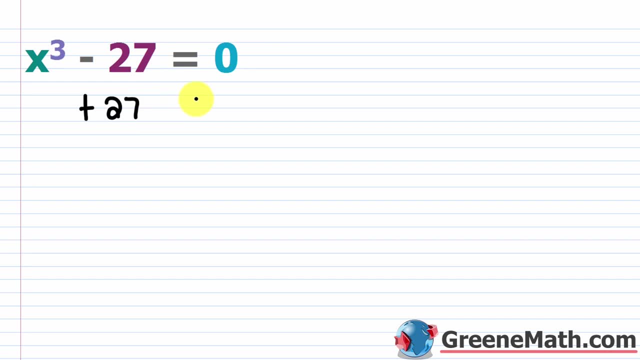 equation like this. Well, the first thing is, I could add 27 to both sides, okay, And I could set this up and say: really, this is x, cubed is equal to 27.. Okay, let's pause and think about this for a 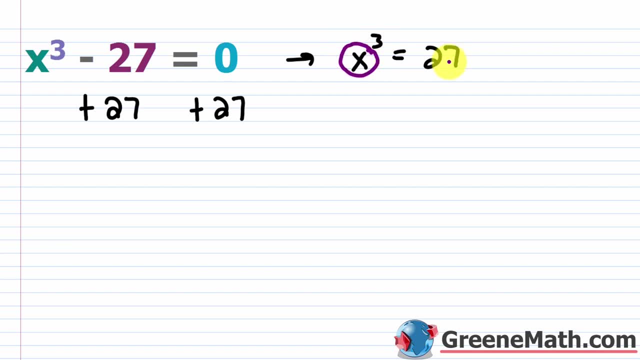 moment. Let's say I have a value that I can plug in here and cube it and get 27.. So in other words, what number cubed gives me 27.? So if I found the three complex cube roots of 27,, I could plug them. 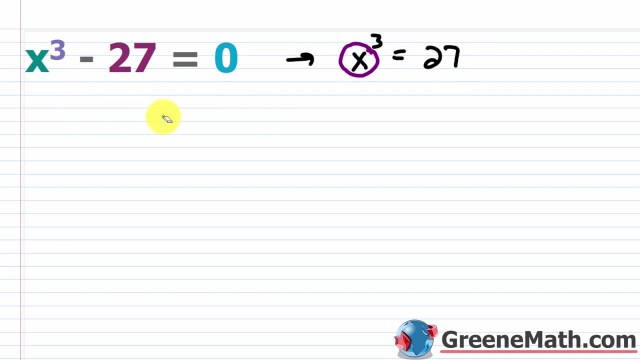 in for x and I would have a true state. Okay, So you might be thinking: well, 27 is a real number. Remember, all real numbers are complex numbers. The real number system is a subset of the complex number system. I can write 27 as 27 plus zero. i Okay. 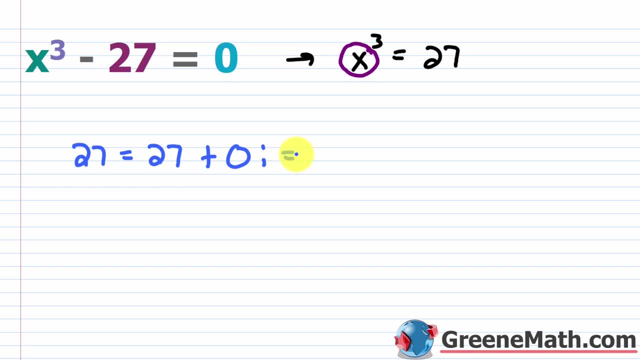 So with this format here, I can also write this in polar form. This is really easy to do. If you think about the r value, it's just going to be 27,. okay, Because you think about this as okay. well, r is equal to the square root of 27 squared. 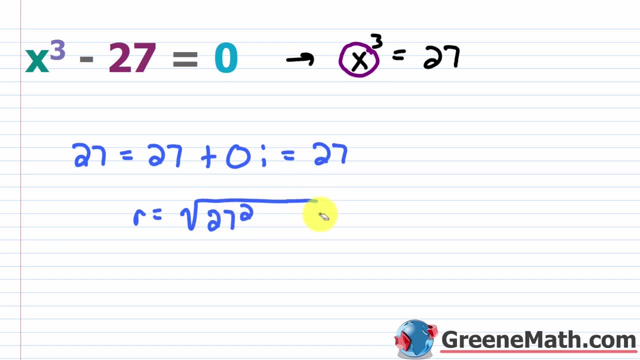 plus 0 squared, 0 squared. you can just get rid of that, okay, And the square root of 27 squared is just 27.. So our r value is 27.. Then, in terms of this inside part, it's easy as well. 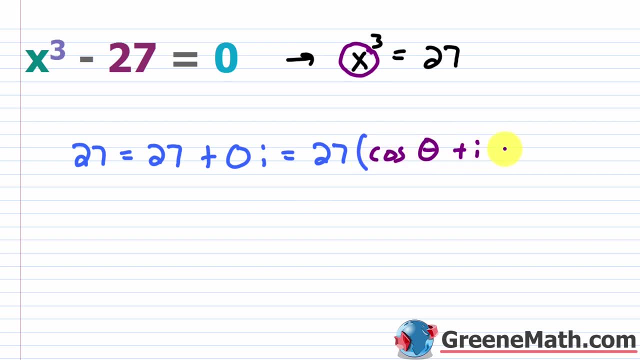 So you'd have the cosine of again theta plus i times the sine of theta, So you don't need to do any inverse tangent function here or anything like that. Just think about this complex number if you graphed it on a complex plane. 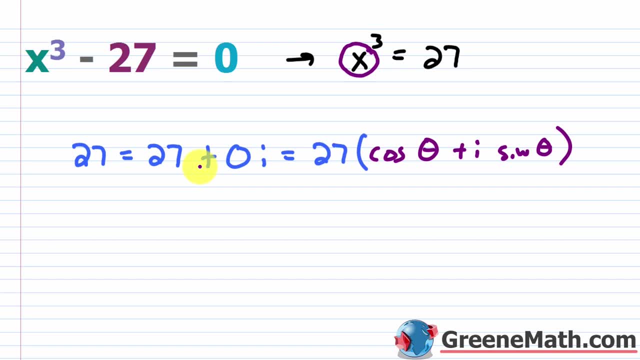 You would simply start at the origin and go 27 units to the right. okay, So there's no movement at all. vertically, right, You're on the x-axis, or the real axis, if you want to think about it that way. So really, this is going to be a zero degree angle, right? 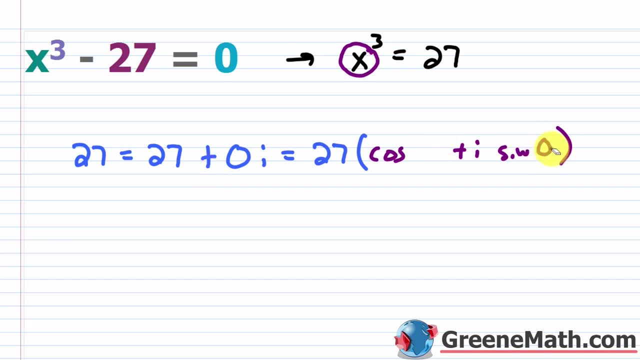 I haven't moved off the real axis, So I'll just go ahead and put this as a zero degree angle. okay, And that's all it is. So this is me writing the number 27,, first in rectangular form and then in polar form. 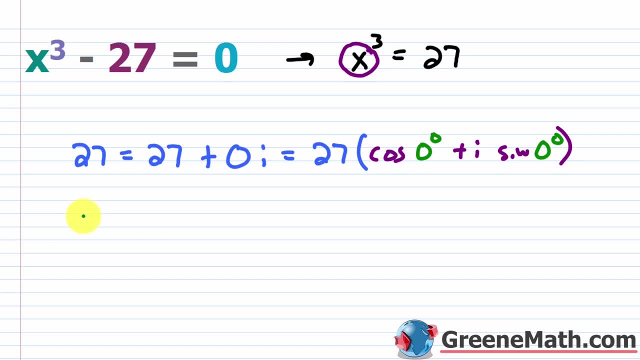 Now, in order to find my three complex cube roots, I'm going to start with my simple little formula. So I have the nth root of r. So in this case, n is 3, right, Because I'm looking for a cube root. 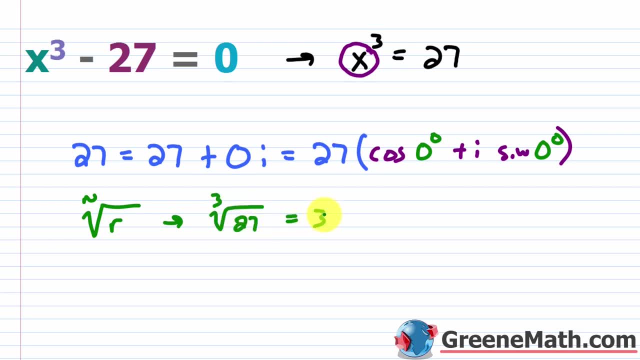 And r is 27.. Well, the cube root of 27 is 3, right. 3 times 3 is 9.. 9 times 3 is 27,. okay, So I can set this up. I know I have three of them. 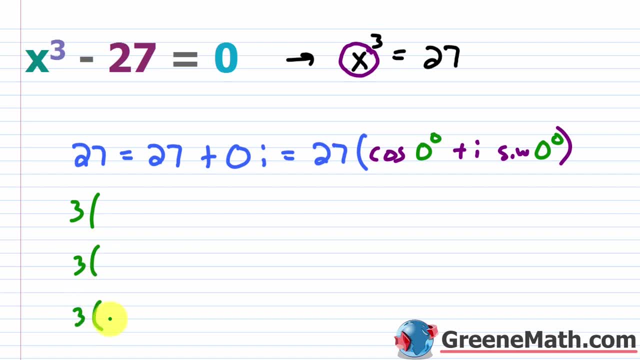 So I'll go 3,, I'll go 3, and I'll go 3,. okay, So let me just write all this out. So we have cosine, cosine and cosine, And we're going to use alpha. We're going to use alpha and alpha. 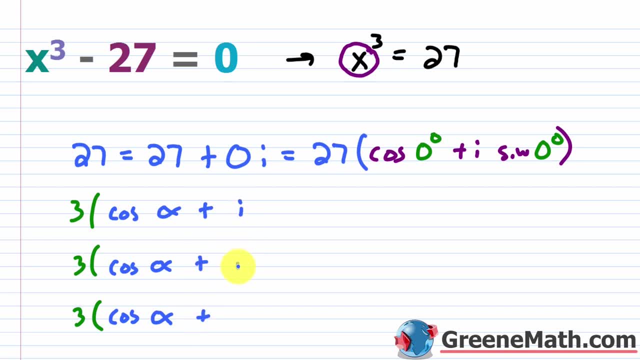 And I'll replace this in a moment. So plus plus and plus I, I and I, And then sine, sine and sine, okay, And I'm going to use alpha again, alpha again and alpha again, okay. 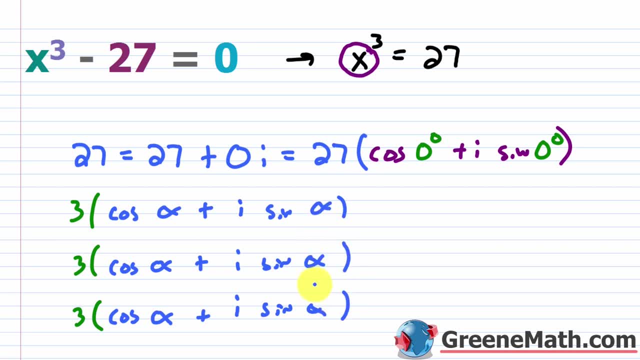 So again, these are all going to change based on that input for k. So to find alpha, let's go ahead and set this up over here. I'll put a little border here To find alpha. the idea is that it's theta, whatever this is. 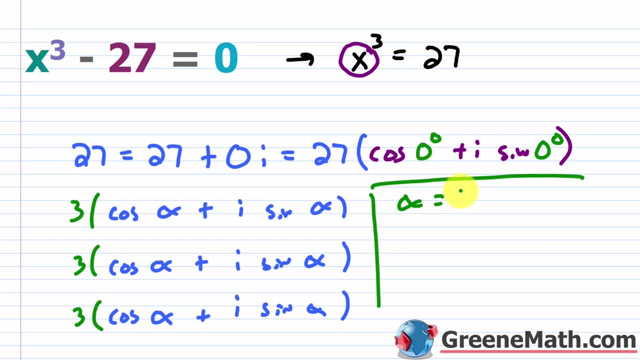 In this case 0.. Degrees divided by n, which in this case is 3, okay, So 0 degrees divided by 3 is just 0 degrees. So this is 0 degrees. You can put it there or leave it off. 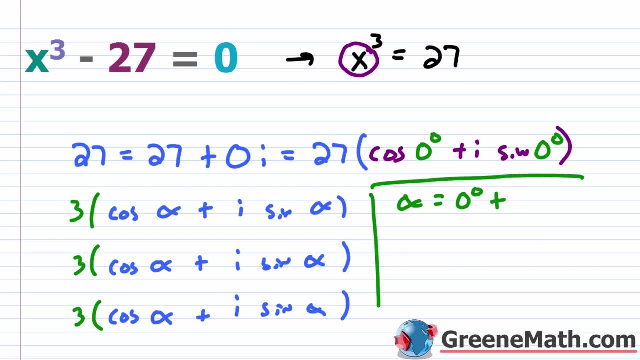 It doesn't matter, It's not going to change anything. I'm just going to leave it for the sake of completeness. So then, plus, you have 360 degrees divided by n. In this case that's 3.. So this is 120 degrees, okay. 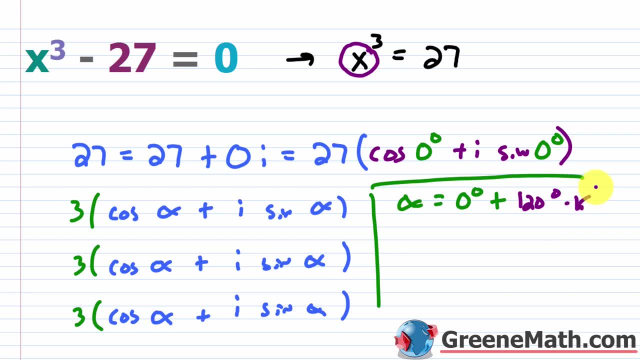 And then times your k. Now k is going to be 0,, 1, and 2.. Basically, your pattern is what It's: 0, comma 1, comma, 2, comma, 3, comma. dot, dot, dot. 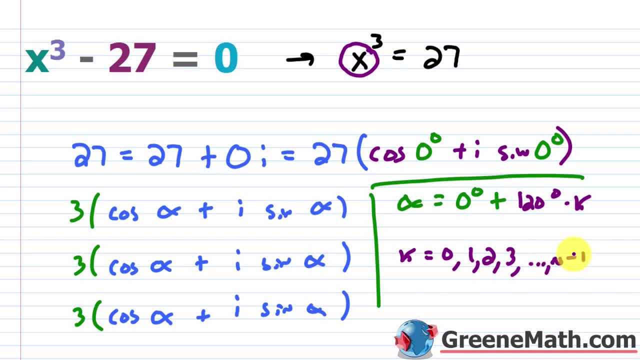 n minus 1.. Let me put a comma in there to make that complete, And basically you have 3.. So 3 minus 1 is 2.. So in this case we would only go up to 2, okay. 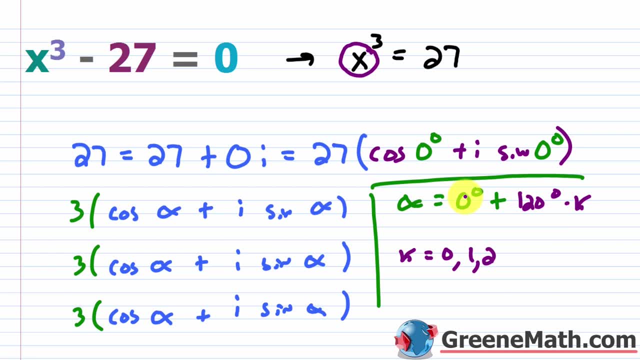 So that's how that works. So I'd start with a 0 there And, of course, 0 degrees plus 0 degrees is just 0 degrees. So the first guy here is just going to be 0 degrees, So I can put that in here and here. 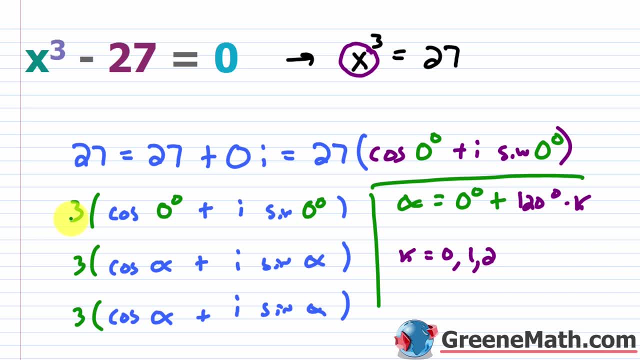 And that should make sense. If I cubed this, 3 cubed would be 27. And then you would basically have 3 times 0 degrees, which is still 0 degrees, and 3 times 0 degrees, which is still 0 degrees. 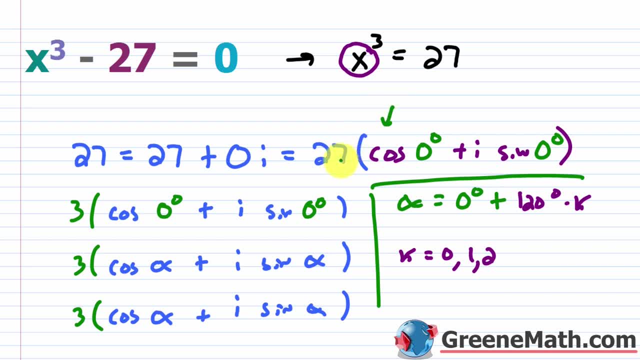 So in polar form- I would be right back to this here- 27 times the quantity cosine of 0 degrees, plus i times the sine of 0 degrees, which, again in rectangular form, is this and written just as a real number, is this okay? 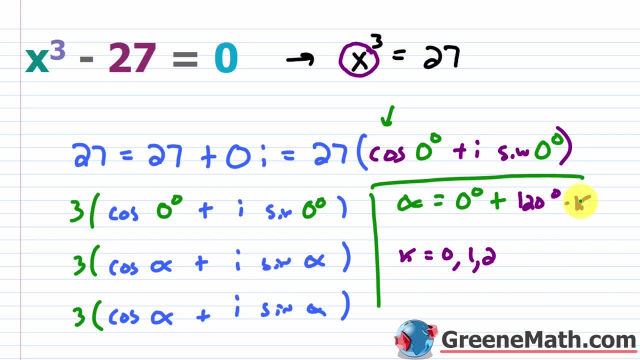 So then the other one. I'm just going to add 120 degrees each time. If I plugged in a 1 there, this would just be 120 degrees. So 120 degrees, 120 degrees, Add another 120 degrees. If I plugged in a 2 there, this would be 240 degrees. 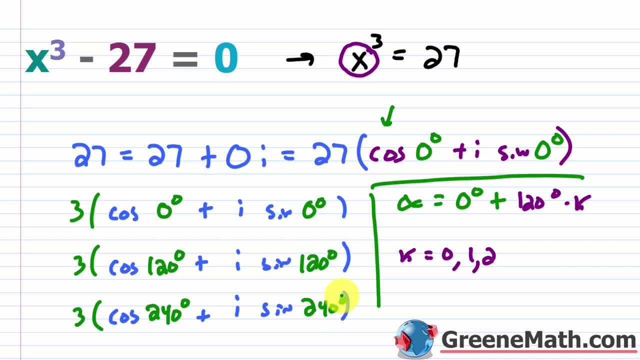 So 240 degrees and 240 degrees. okay, So these three numbers here in polar form, these three complex numbers in polar form, if you cubed them, they would each give you 27.. Now, typically, if you were in an algebra class, you would not give this as your solutions, right? 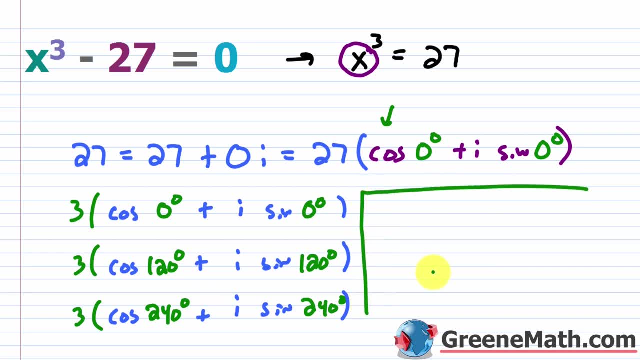 You would want to convert this back into rectangular form. okay, So how would we do this? The cosine of 0 degrees is going to be 1, and the sine of 0 degrees is going to be 0. So basically, you would have 3 times 1, which is 3.. 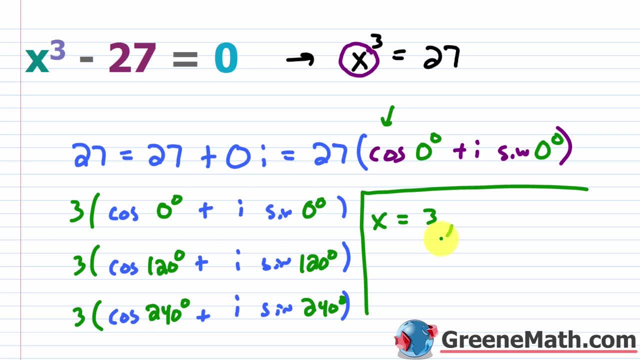 So I would say x is equal to 3,. okay, That would be my first solution For this one. the cosine of 120 degrees And the sine of 120 degrees. let's think about this. There's a 60-degree reference angle here, here, here and here, right. 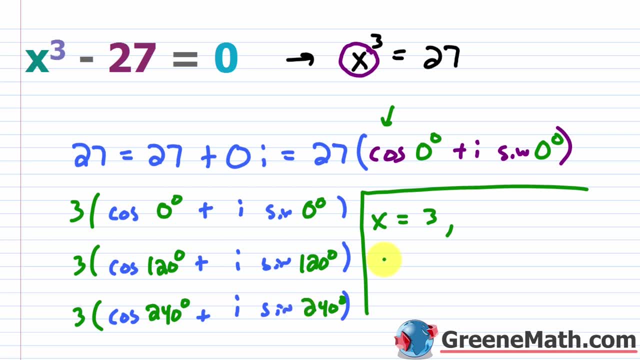 120 degrees, 240 degrees, you have a 60-degree reference angle. So the cosine of 60 degrees is going to be 1: half And the sine of 60 degrees is square root of 3 over 2, okay. 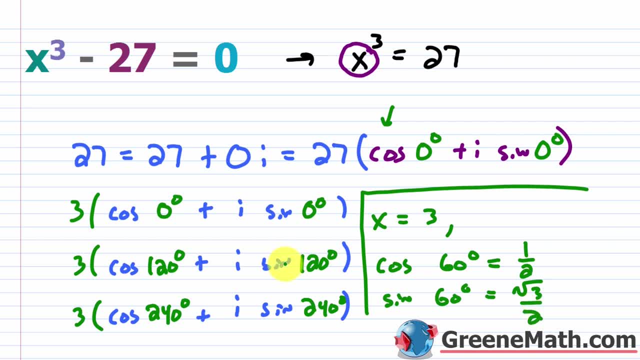 So it's just a matter of getting the sines right. Remember, sine is going to be positive in quadrants 1 and 2, and 120 degrees is in quadrant 2.. Cosine is going to be positive in quadrants 1 and 4, okay, 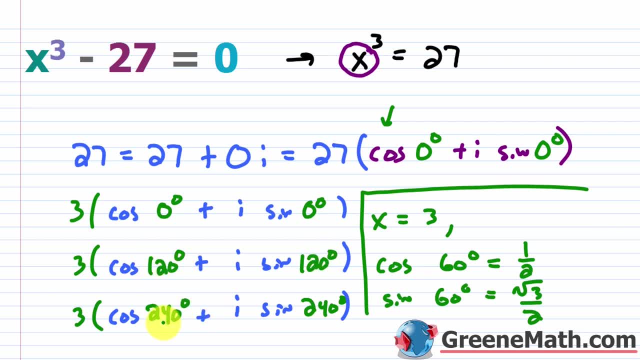 So, basically, So basically, cosine is negative in each case, because this is quadrant 2,, this is quadrant 3, and sine is positive here and negative here. okay, So to get my solutions, let me write this out. I'm just going to scroll down a little bit so we have some room. 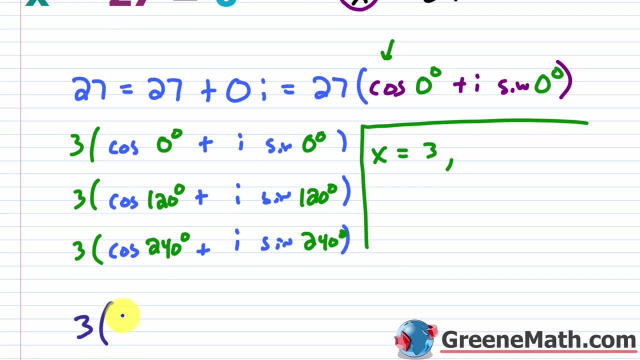 For this one I would have what? 3 times this would be the quantity negative: 1 half plus this guy is going to be square root of 3 over 2, okay times i. So if I go ahead and distribute the 3 into each term. 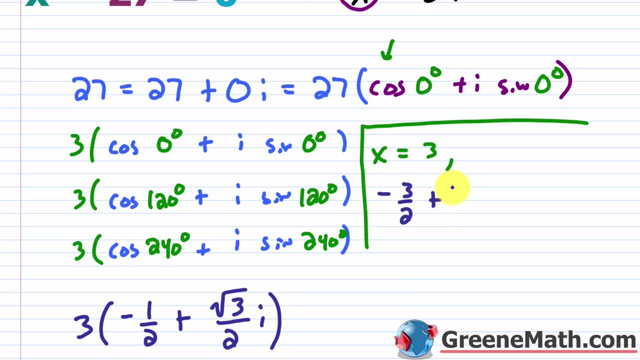 I would have negative 3 halves and then plus my 3, times square root of 3 over 2, times. i okay, So that's another solution. Then the other one. let me just go ahead and keep this as negative. 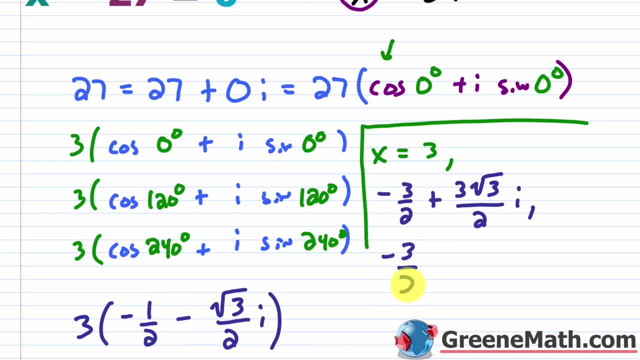 and I'm going to change this to negative now. So basically you would have negative 3 halves again, and then minus the 3,, minus the 3, times square root of 3 over 2, and then times i okay. 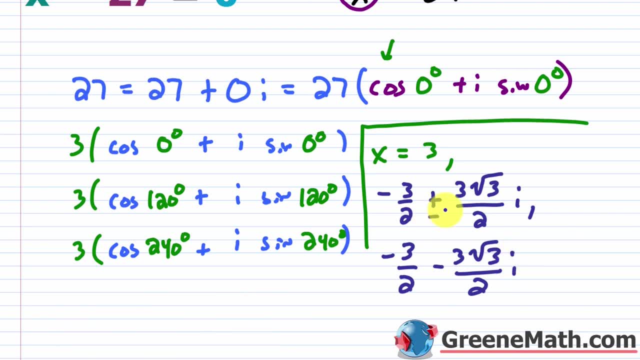 So I would write this in a more compact form. I would just do plus or minus here and get rid of this. That way you can more cleanly write your three solutions. So if you were in an algebra class and they gave you this equation, 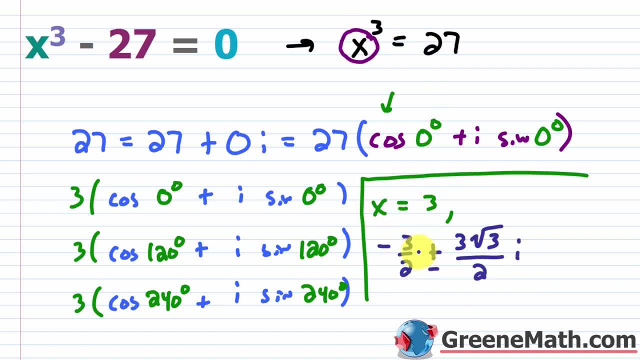 you would want to give this as a solution. Now, in this particular case, this is probably not the fastest method to do this, but it's one such method that you can get a solution. Now, let's think about this graphically. If I wanted to show these solutions again, I'm going to do this in polar form, okay, 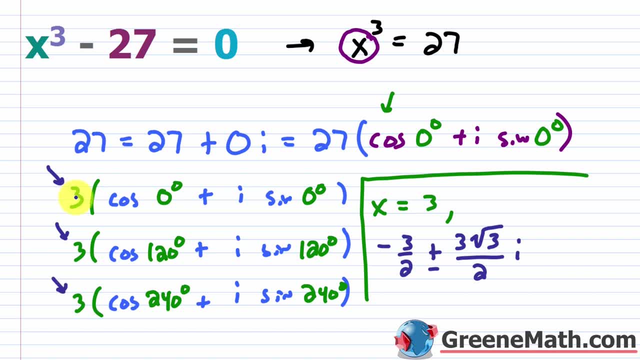 So on the Argand diagram or the complex plane, again the magnitude is 3 in each case, So that's the length of your vector. So if you're making a circle, okay, with a radius of 3, that is centered at the origin. 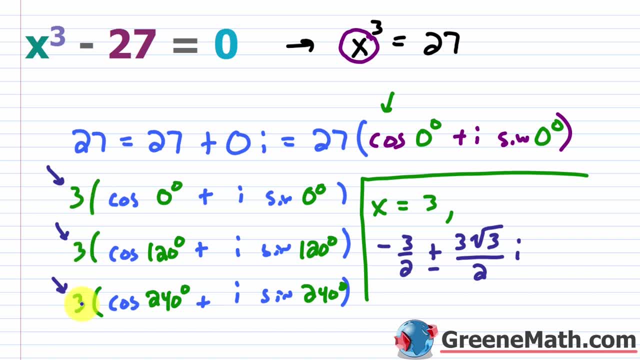 each one of these vectors is going to touch that circle. okay, That's going to be your terminal point. that lies there. Okay, Then your direction angle for your vector is going to be 0 degrees, then the other one's going to be 120 degrees. 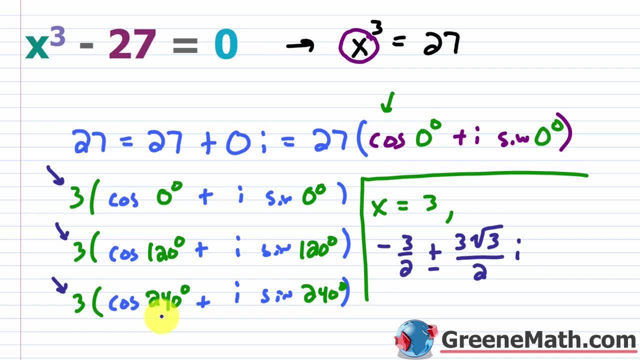 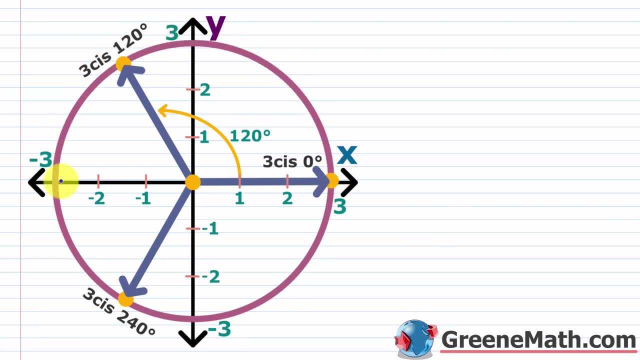 then the other one's going to be 240 degrees. okay, All of them are position vectors, so they start where their initial point is, at the origin. So, graphically, this is a rough sketch of this guy. Again, I have a little circle that's drawn. 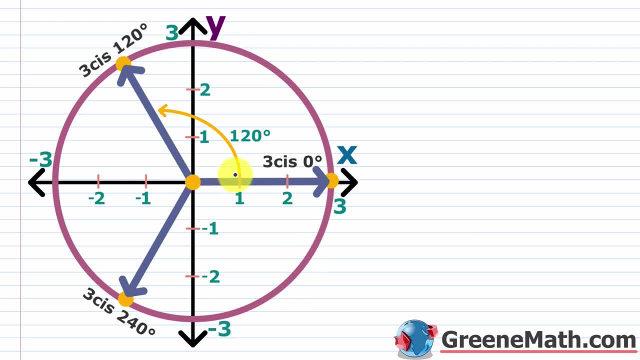 and the radius is 3, and the center is at the origin. okay, Then you have your three position vectors. Notice that they're all going to have an initial point at the origin. The terminal point in each case is on that circle. 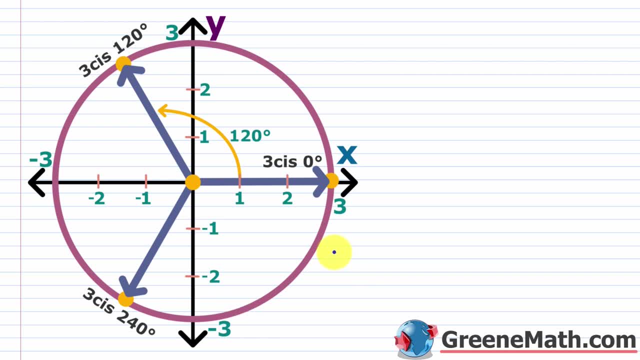 again, where the radius is 3, and the center is at the origin. So your first angle is 0 degrees. okay, It's given by this 3, cis 0 degrees. Again, this is the abbreviation. The second angle is 120 degrees. okay. 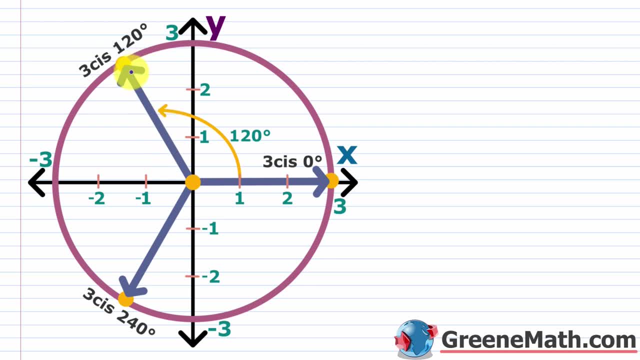 So we come from here, we rotate 120 degrees and now we have that vector there, okay, And the terminal point's there, And then the last one. if I rotate around here, this is going to be a 240 degree angle, okay. 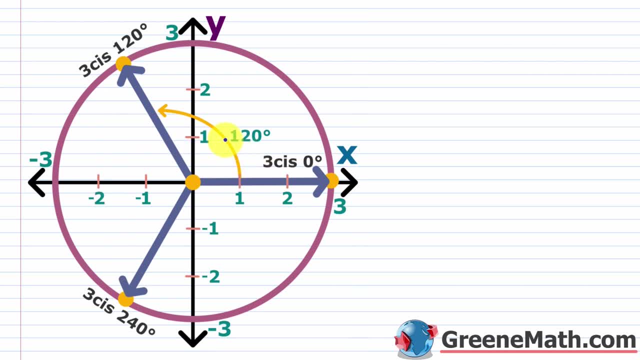 So that's how you would sketch the graph of this guy. You'll notice that these guys are equally spaced 120 degrees apart. right, 120 degrees. this is 120 degrees and this is 120 degrees as well. So this is how you can graph your solutions, if you're asked to do them. 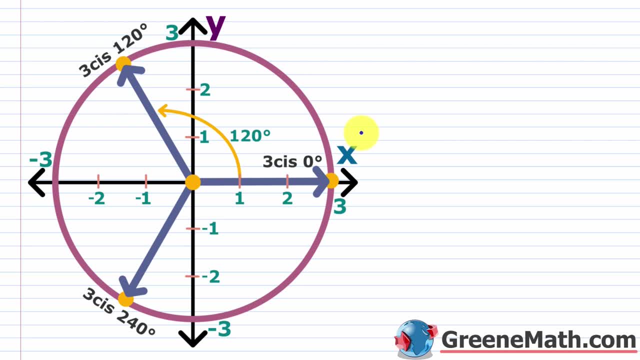 Again, figure out the magnitude or the length of the vectors. You're going to sketch yourself a little circle, okay, With a radius of that number- in this case it's 3, and a center at the origin. So all of your vectors are going to be position vectors. 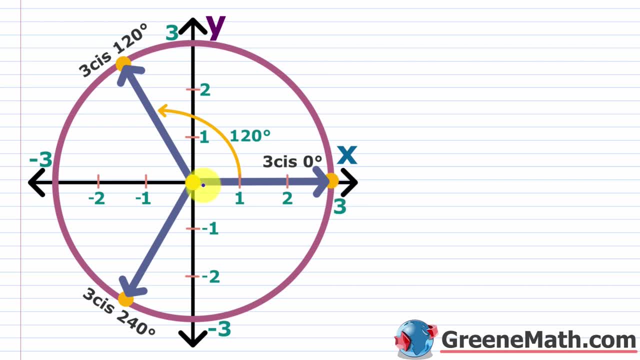 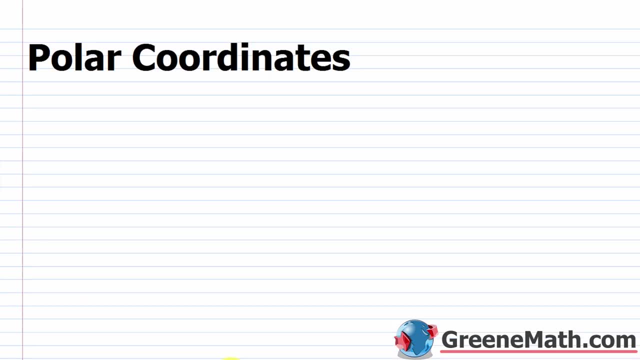 initial point at the origin. terminal points can be on that circle and you just get your direction angle from your roots. So we had 0 degrees, 120 degrees and then 240 degrees. In this lesson we want to talk about polar coordinates. 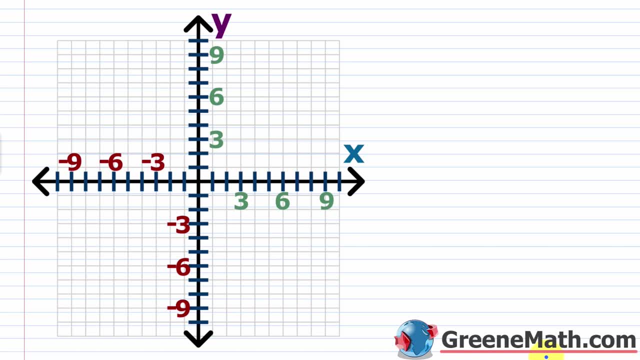 All right. so up to this point, we've exclusively used something called the rectangular coordinate system, or some people refer to this as the Cartesian coordinate system, after the inventor, And we've worked with this guy to plot these points, or you could say ordered pairs. 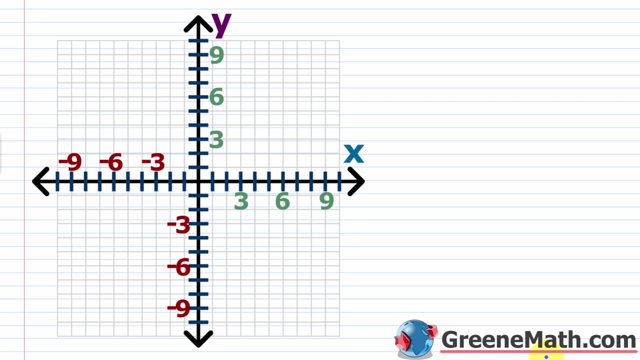 and also to graph equations. So I want you to recall that the rectangular coordinate system is going to feature the x-axis, which is horizontal, and the y-axis, which is vertical. Okay, the meeting point between the two is going to be right here. 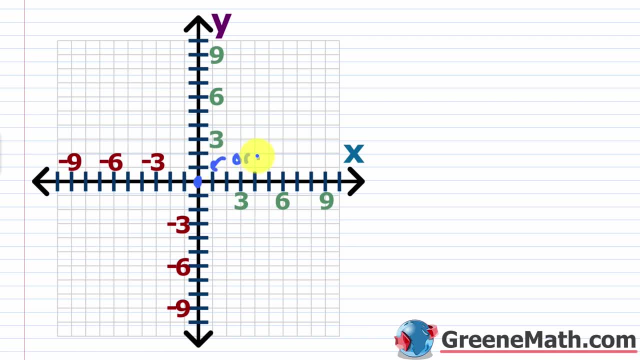 and this is referred to as the origin. Okay, so this is your origin or origin? okay, And when we specify this using an ordered pair, remember this is the x-value comma, the y-value, So for the origin it's going to be 0 comma 0, okay. 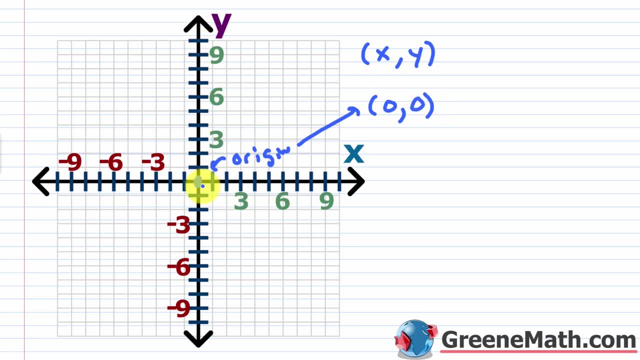 Because the x-value is 0, and the y-value is 0. Now, if I think about another point, let's just do a few. So let's say we do something like 6 comma 7.. Let's say we do negative 6.. 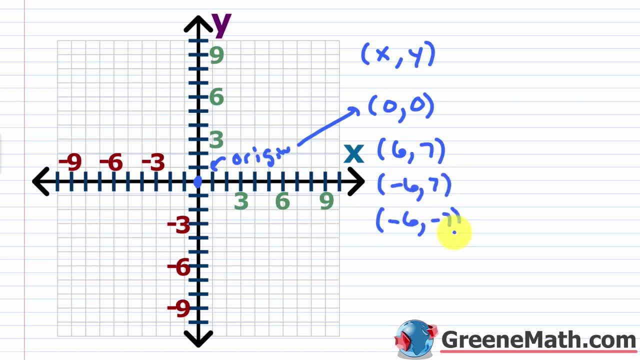 Let's say we do negative 6.. Let's say we do negative 6.. 6 comma 7,. let's say we do negative 6 comma negative 7, and let's say we do 6 comma negative 7, okay. 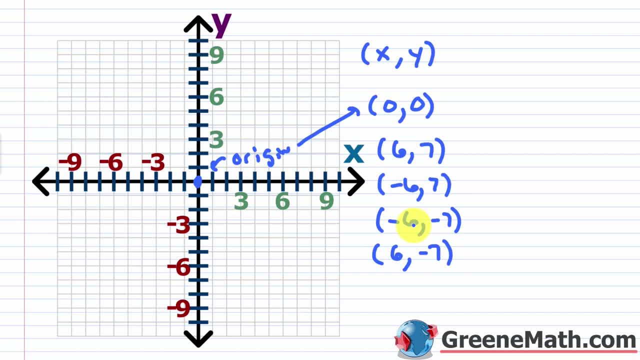 So these are directed distances, okay, from the origin. So, in other words, the first guy here, okay, or the first component, as they say, the x-value tells you how to move horizontally. okay, If it's positive, I'm moving to the right. 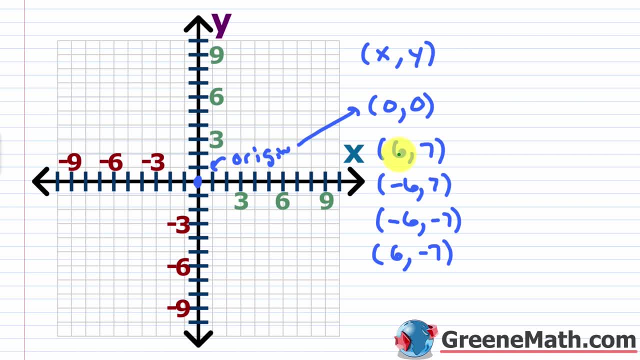 If it's negative, I'm moving to the left. So for this guy, 6 comma 7, I'm moving to the right by 6 units. Okay. so let me just circle this temporarily. And then the second guy there, the y. 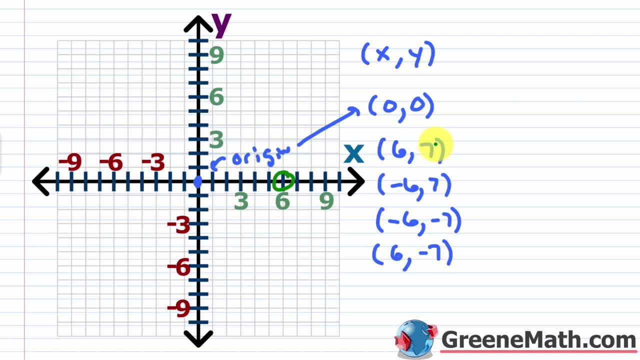 the coordinate is telling me how much to move vertically right. So if it's positive, I'm going up, If it's negative, I'm going down. So let me go ahead and, from the origin, go up by 7 units. okay. 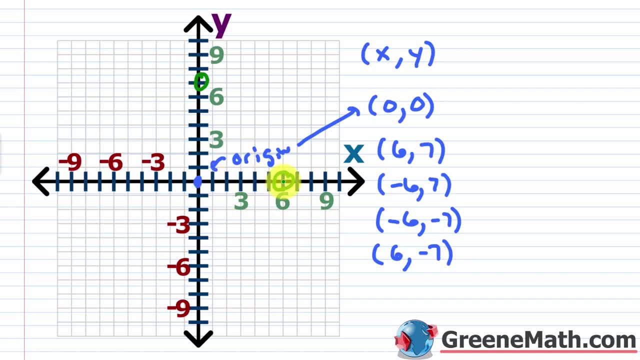 So you basically want the meeting point between the two. So you can go 6 units to the right and 7 units up, or you can go 7 units up and 6 units to the right. okay, Either way, you're going to end up at this point, right here. 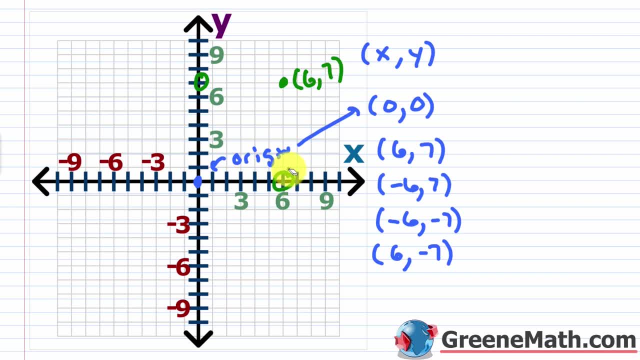 This is going to be your 6 comma 7.. And I know most of you know how to do this already, but basically we just want to recap this before we get into the polar coordinate system. Now for the next one. we have negative 6 comma 7.. 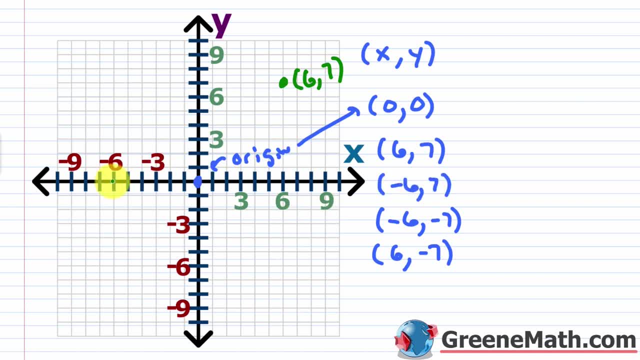 So that means I'm going 6 units to the left right because it's negative 6.. And then I'm going 7 units up because it's positive 7, okay, So 6 units to the left, 7 units up. 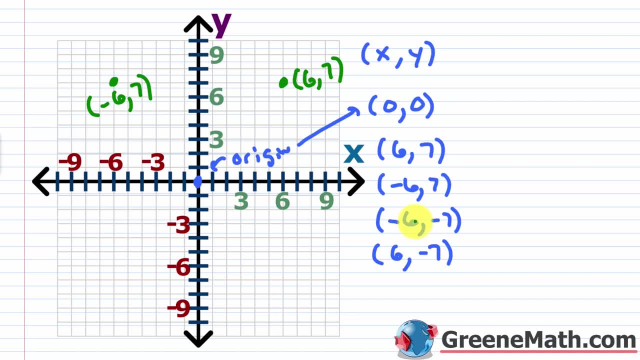 So this is my negative 6 comma 7, okay. The other one is negative 6 comma, negative 7.. So both are negative. So it means I'm going to the left, okay, because it's a negative 6. And I'm going down because it's a negative 7.. 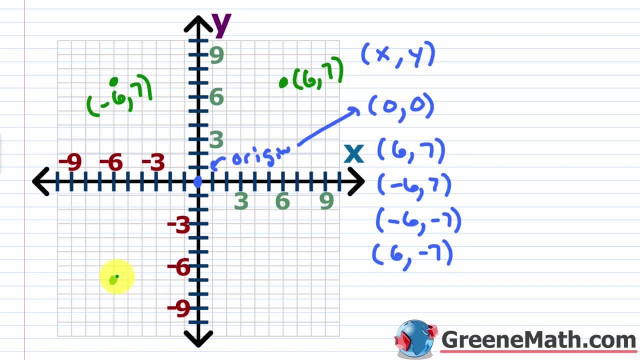 So 6 units to the left and 7 units down. That's going to put me right there, okay. So this would be negative: 6 comma negative 7.. And then, lastly, we have 6 comma negative 7.. So this is positive for x and y is negative. so it means I'm going to the right and I'm 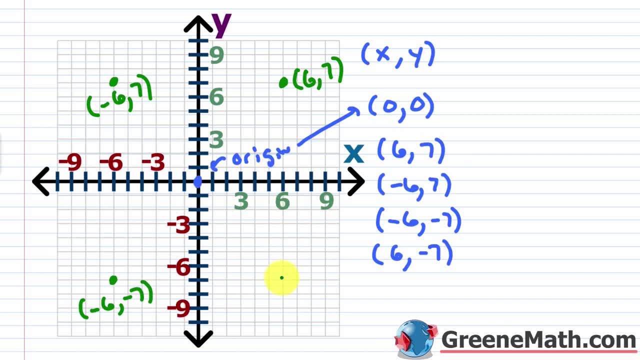 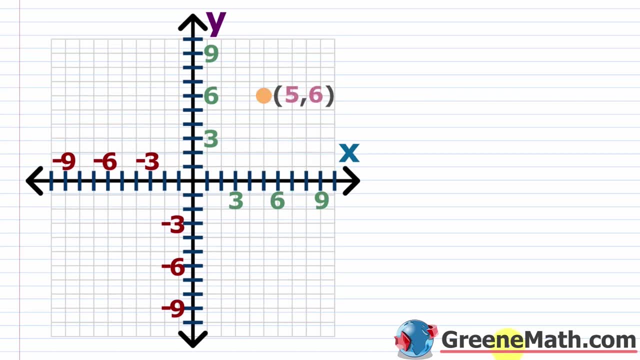 going down right. So 6 units to the right and 7 units down. That's going to put me right there, okay, So this is 6 comma negative 7.. All right, now let's think a little bit about something called the polar coordinate system. 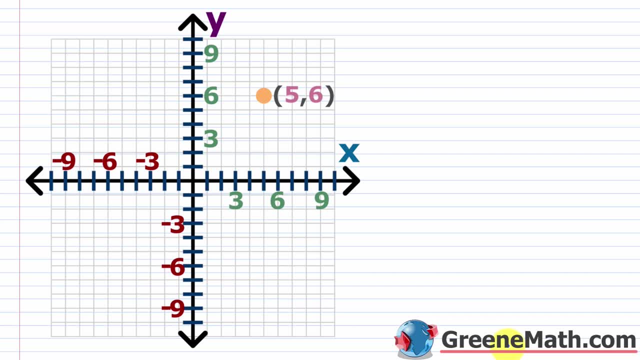 And to start this out, I'm just going to show you how we get the polar coordinates. So let's say I had something like the point where we have 5 comma 6.. So this is as an ordered pair. again, this is x comma y. 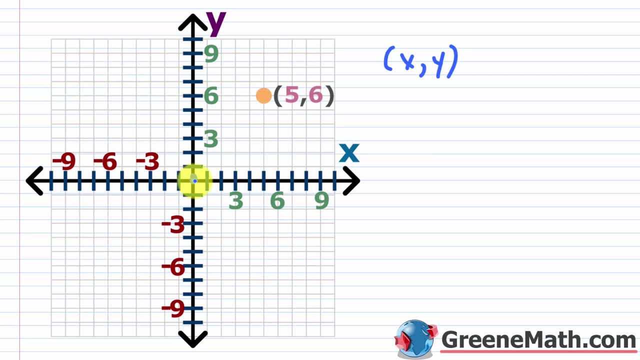 So, starting at the origin, I know that to get to this point I could go 5 units to the right and 6 units up, So that puts me right there. Or, alternatively, I could start at the origin and go 6 units up and 5 units to the right. 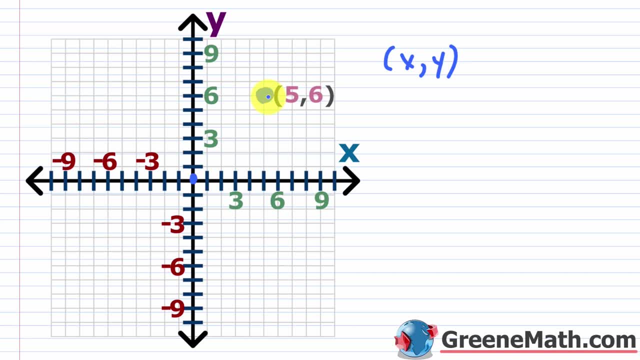 So, basically, that gives me the directed distances from the origin. We know that, But we also want to be able to write this with polar coordinates, which is going to be an r value, comma, a theta value, okay, So where does this come from? 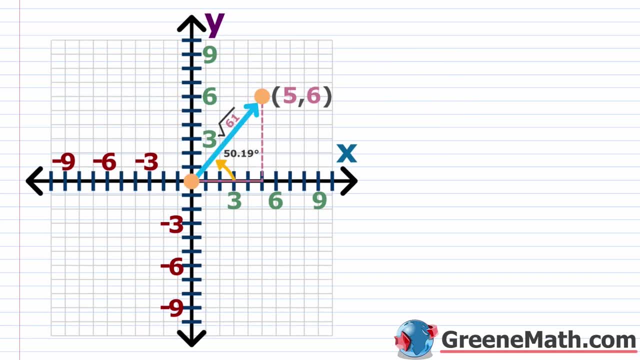 Well, essentially what we can do is we can create a little position vector, Okay. So the initial point is at the origin. The terminal point is going to be at that point here. okay, with our 5 comma 6.. So what I could say here is that with rectangular coordinates you have x comma y. 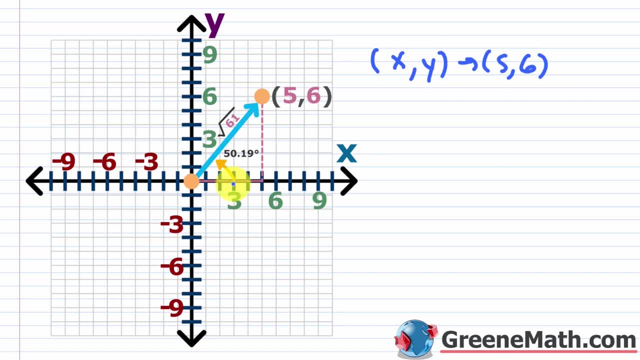 In this case it's 5 comma 6.. So, hey, start at the origin, go 5 units to the right and 6 units up. With polar coordinates, it's going to be r comma theta, okay, where r is the distance. 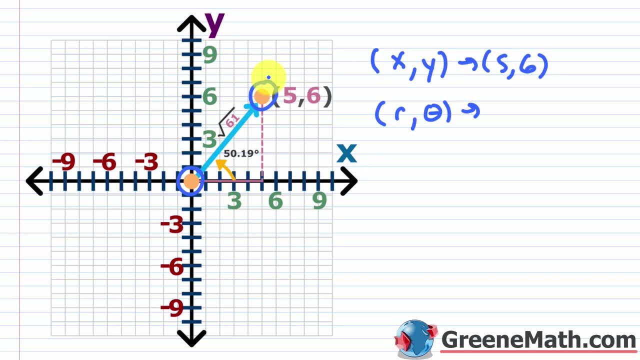 from here to here. Okay, If you're thinking about this as a vector, remember the length of the vector is called the magnitude of the vector, So in this case, that's going to be your r right. So this is the square root of 61.. 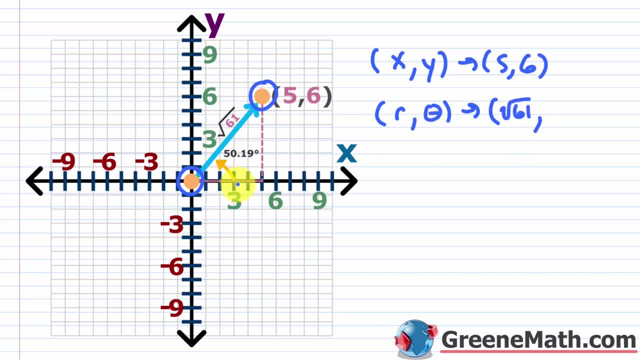 And then the theta here is the directed angle. So, in other words, how much do I need to rotate counterclockwise? So, starting from the positive x-axis, if I'm facing this way, I need to rotate by 50.19. 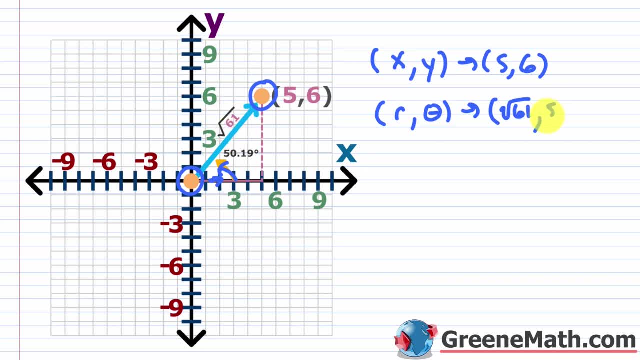 degrees to get to this position vector. okay, So let's say this is 50.19 degrees. This is an approximation and I'll talk about how to get this in a moment, But essentially I want you to see that it's just two ways to get to the same point, right? 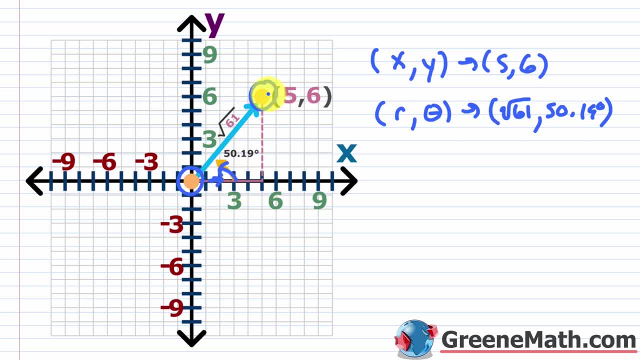 I can't get to the same point. I could say, hey, start at the origin, go five units to the right and six units up. Or I can say, hey, start at the origin. okay, facing the positive x-axis rotate 50.19 degrees. 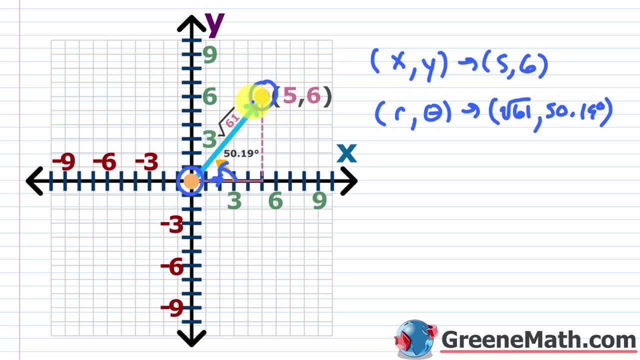 and then walk forward by the square root of 61 units. okay, So two ways to kind of do the same thing. Now, if we want to talk a little bit about where this r value came from and where the theta value came from, see here how I made a little right triangle okay. 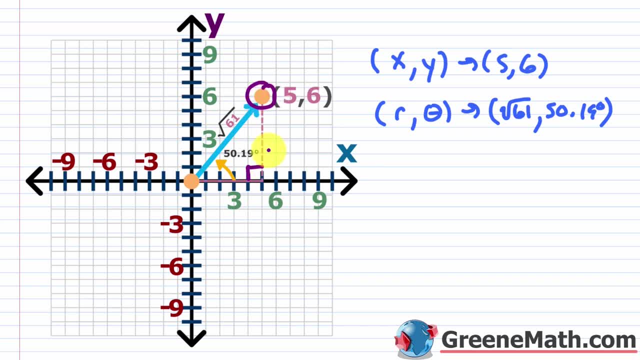 And essentially we see that the length of this vector is going to be equal to the length of this vector. This vertical leg here is given by the y value of six right. So this is basically from zero to six. so this is given by six. 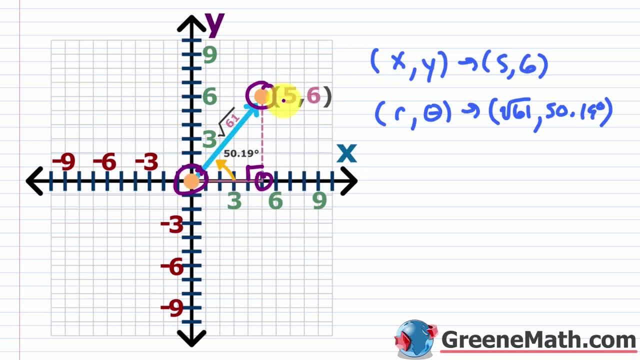 The length of this horizontal leg here is given by the x value of five. okay, So really easy to work with this. You just use the Pythagorean theorem. So, if you want your distance from here to here or the magnitude of the position vector, 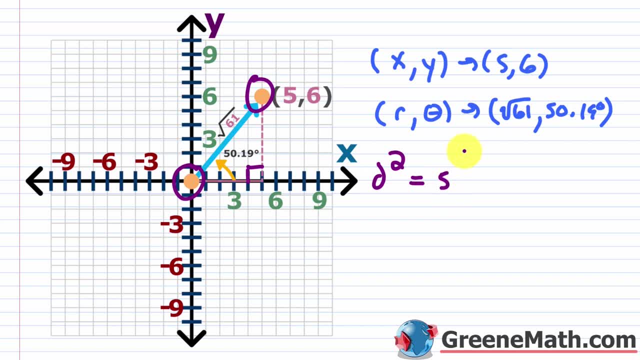 the distance squared would be equal to. you would have five squared, and then plus six squared, So d. your distance between these two points would be equal to the square root of 61.19, right, So d would be equal to the square root of five squared is 25, plus six squared is 36.. 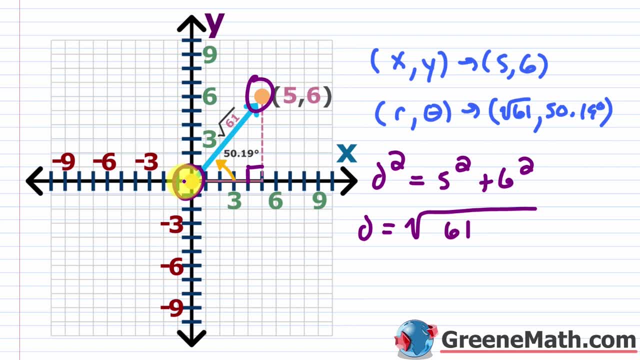 If you sum those two together, you're going to get 61, okay, So the distance between these two points, or your r value, is a square root of 61, okay, So that's where that came from In terms of theta. okay, calculating that, basically, for most textbooks they're going. 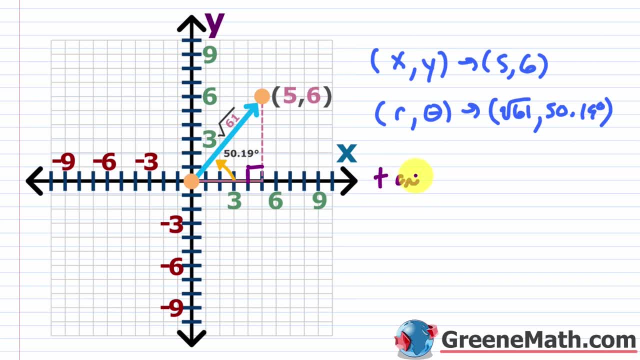 to use the inverse tangent function. Remember the tangent of some angle theta is y over x. okay, So in this case, your y value is six, Your x value is five. So let's go ahead and say that the tangent of theta is six over five. okay, 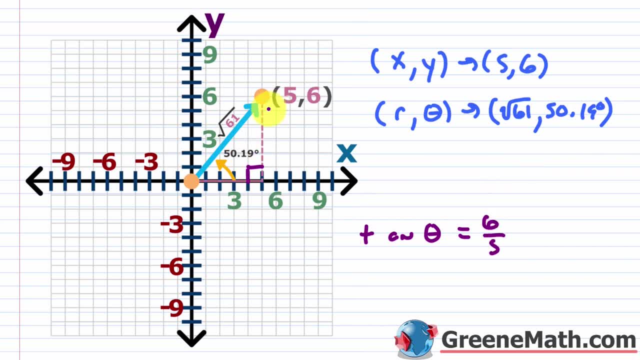 And then, because we're in quadrant one here, we can go ahead and just strictly use the inverse tangent function, right? So I can just say the tangent inverse of six fifths, like this, is going to give me- and this is an approximation, so we'll say- approximately 50.19 degrees. okay, 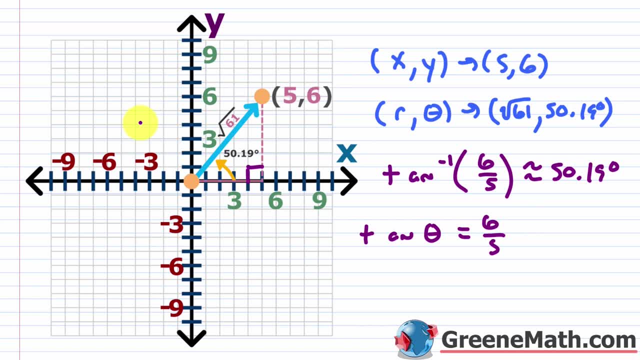 Now, if you're in another quadrant, you have to be really careful because, remember, the inverse tangent function is only going to give you something. in quadrant one, okay, if this argument is positive. or in quadrant four, rotating clockwise, if this argument. 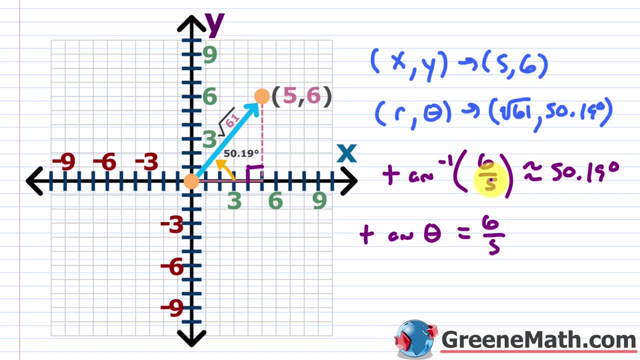 is negative, So be really, really careful. We're going to work a lot of examples today, and I'll show you how to deal with that. All right now. what I want to do is just take you through the basics of the polar coordinate. 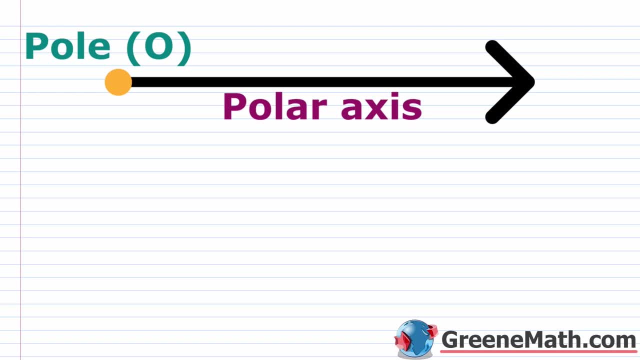 system. So with the polar coordinate system, everything is going to be based on a fixed point, which is called the pole or the origin. okay, And essentially most books are going to name this with a capital letter: O. So this is our pole. okay, to get things started. 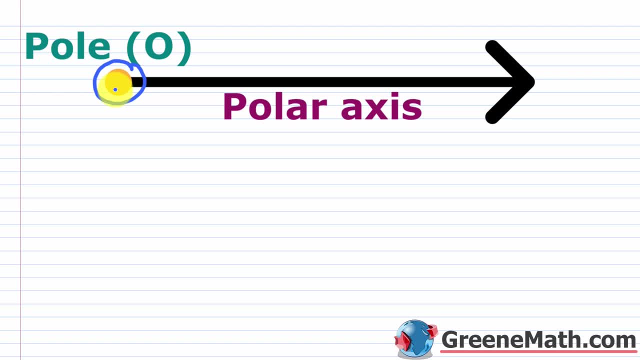 From there you're going to create an initial ray which is called the polar axis. So that's going to be this guy right here. okay, so that's your initial ray called the polar axis, And, generally speaking, this is drawn in the direction of the positive x-axis. 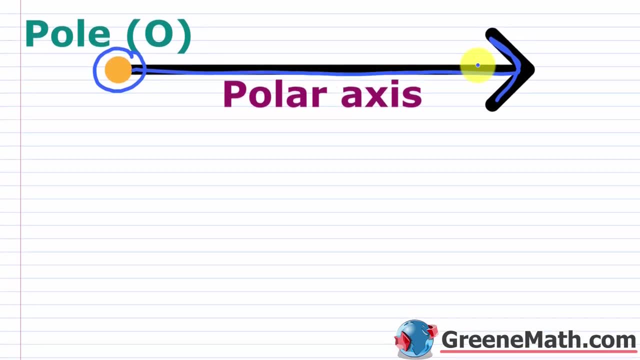 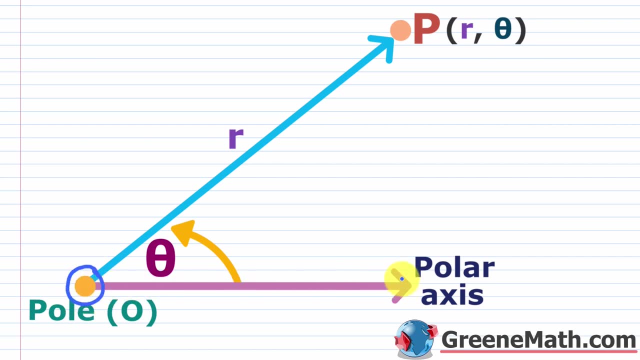 Now, once we have this set up, we can find a point P in the plane using the coordinates r comma theta. okay, So we have our pole here. okay, that's set up. We've constructed the polar axis. So now, if I give you r comma theta, I can locate any point P, okay. 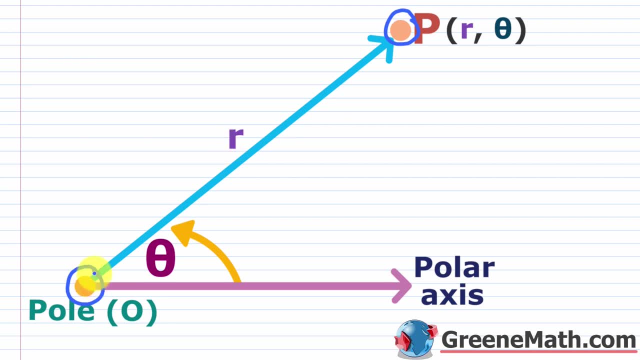 So r is the distance from the pole O- okay- to that point, P- okay. So basically, if you think about this as the vector OP, what is the magnitude of that vector? okay, That's going to be r. And then, if I think about my directed angle, theta, well, this is just telling me how much. 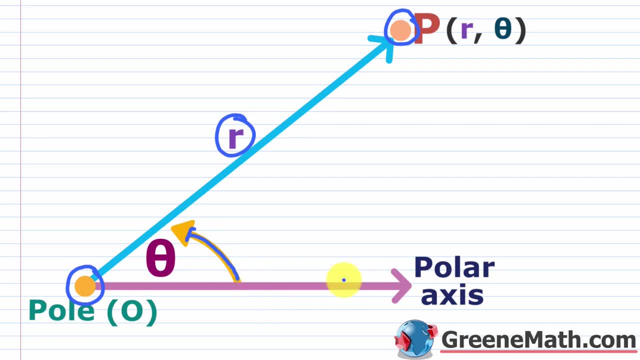 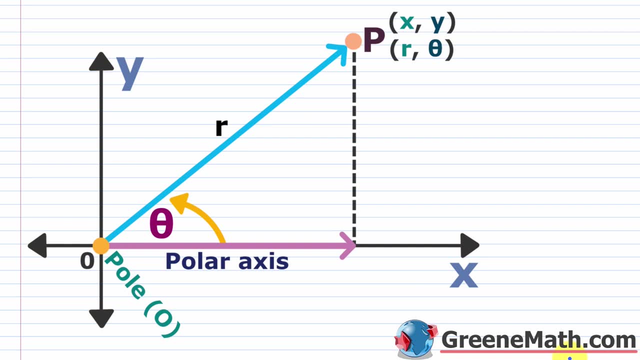 do I need to rotate counterclockwise from the polar axis to get to this vector OP? All right, So what I want to do now is talk a little bit about how to convert between the polar coordinates and the rectangular coordinates. So what we did here is we just took the drawing from the last section, okay, and we just put. 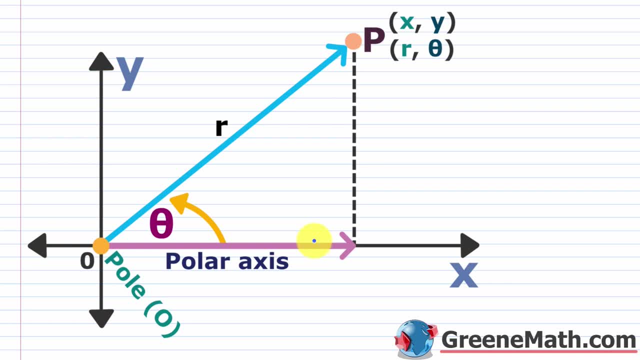 it on top of, basically, a coordinate plane that we're used to right, So the rectangular coordinate plane. You'll see that we have the pole that's going to be fixed at the origin of the Cartesian coordinate plane And basically the polar axis is drawn to coincide with the positive x-axis. okay, 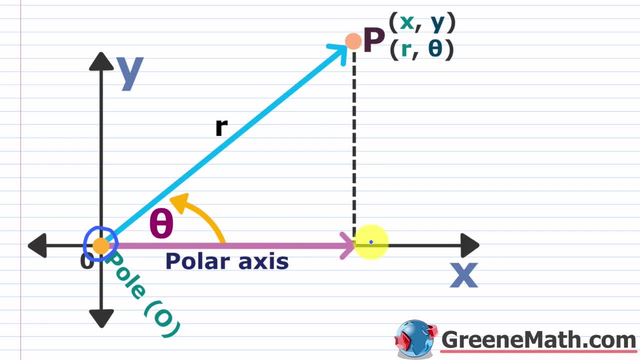 So, In order to do this, we can obtain a few insights here. okay, So we have this point P in our plane, which can be assigned the rectangular coordinates x comma y or the polar coordinates r comma theta. So let's say I gave you r comma theta and I said, hey, I want you to give me x comma. 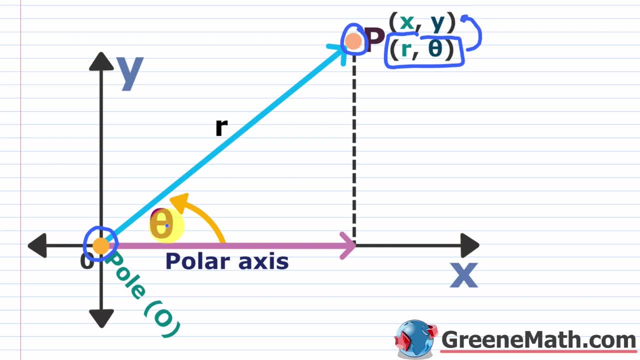 y. How could you do that? Well, if you consider that the cosine of theta is equal to what Remember, I've formed a little right triangle here, so essentially I can say that it's going to be the adjacent which is going to be x-axis. 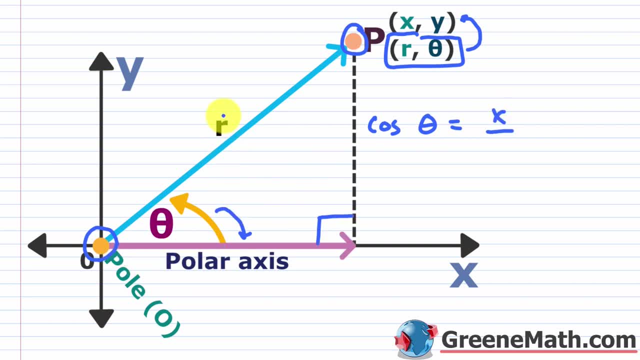 Okay, So it's going to be x here. okay, Over the hypotenuse which is going to be r here. Okay, So x over r, And then, if I think about the sine of theta, it's the opposite, which is y over the hypotenuse. 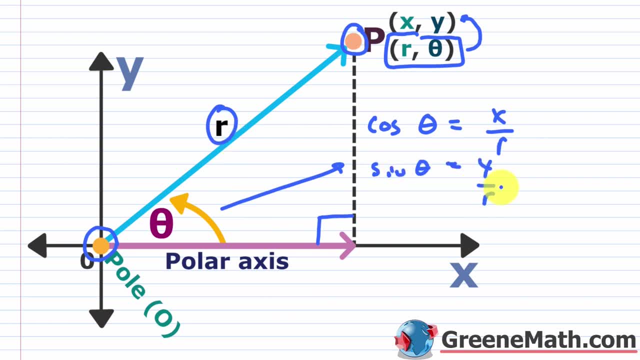 which is r. So the sine of theta is y over r, And I didn't make the equal sign very good. okay, In each case, I can multiply both sides by r. I can solve for x or y. okay, So I can say that x is equal to r times. cosine of theta. 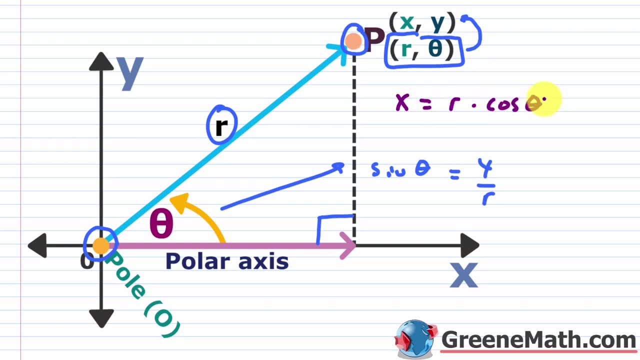 So x is equal to r times cosine of theta, Okay. And then for y, it's going to be r times sine of theta, okay. So y, y is going to be r times the sine of theta, okay. So pretty easy to go from polar coordinates to rectangular coordinates. 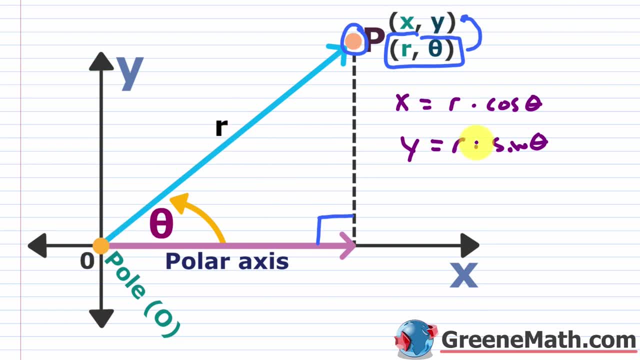 Now let's erase this and let's consider the other one, which is a little bit more involved. But basically, if I start with my rectangular coordinates- my x comma y- and I want to go to my polar coordinates- r comma theta- let's think about that. 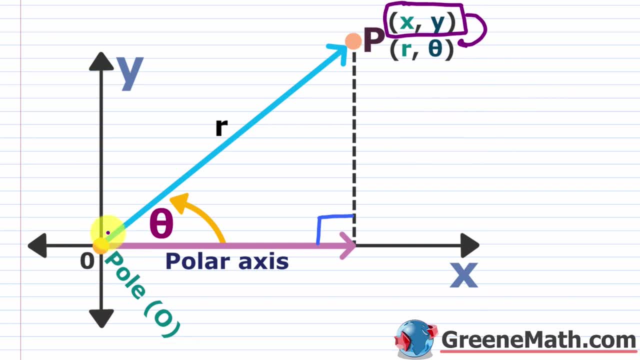 So, essentially, what I'm doing here is: I'm again, I'm going to go to my polar coordinates: r, comma, theta. Let's think about that Again, returning to the fact that for r, I want the distance from here to here. okay, 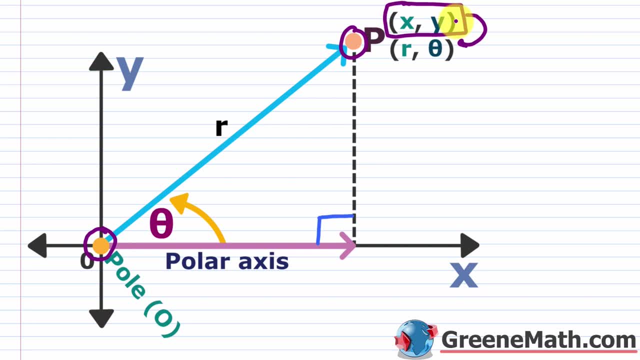 So if I'm given the x comma y again- I'm just using the Pythagorean theorem- r squared is going to be equal to x squared plus y squared. So r is going to be equal to the square root of x squared plus y squared. okay, 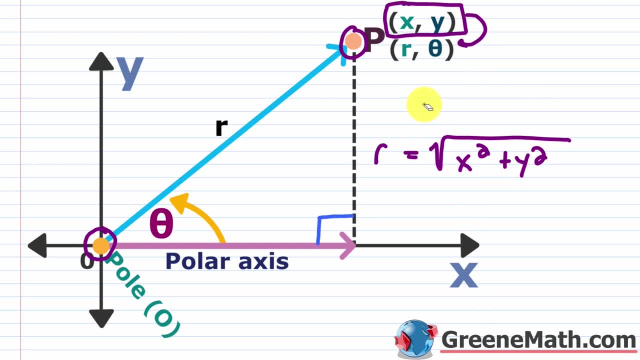 That's all. it is So very easy to remember this. Now the tricky one is to get theta right, Because you have all these different scenarios you have to consider. If you're in quadrant one, you can just use your inverse tangent. 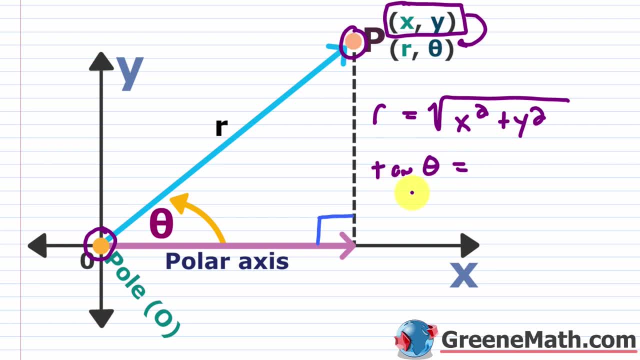 Right, Because the tangent of theta is what It's going to be: y over x. We know this already, But if I'm not in quadrant one, then basically I need to get a reference angle. okay, using the inverse tangent function. 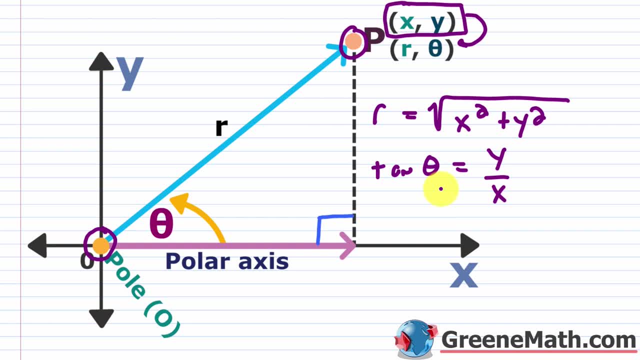 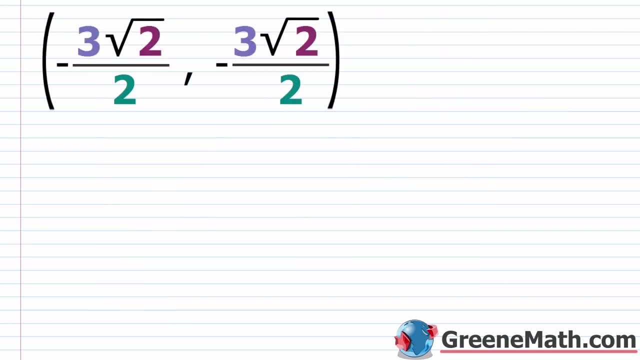 And then from there, I need to take the appropriate action based on what quadrant I'm in, right, So if I'm in quadrant two, three or four, okay, So let's go ahead and think about a simple little example. And so what I have here is the negative of three times square root of two over two, and 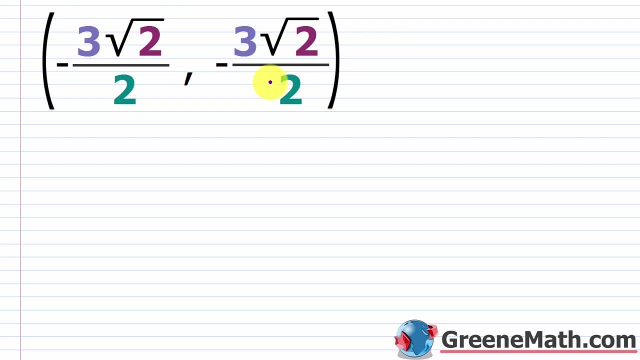 then comma Negative of three times square root of two over two. okay, So these are rectangular coordinates. I want to go to polar coordinates and then I'm going to show you how to plot this on the polar grid. okay, So essentially, this is again my x value and this is my y value, okay, 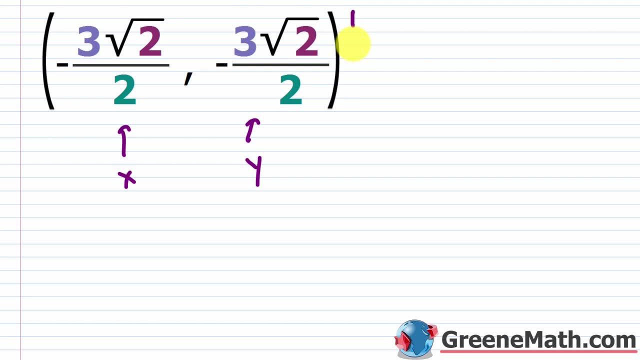 So what did I just say? Essentially, if I want to find the r value, the r value is going to be the square root of x squared plus y squared. okay, So that's the first thing I would do. So all I need to do, let's go. the square root of I'll put r out here is equal to I'll. 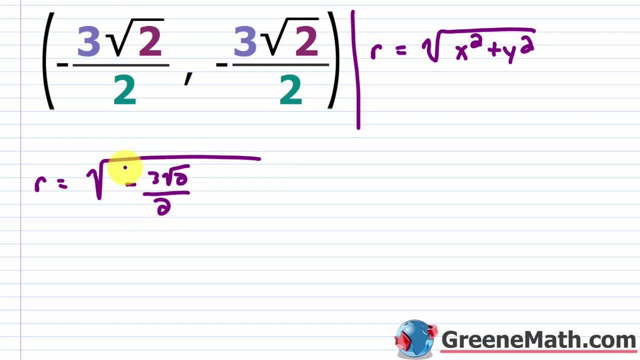 have the negative of three times the square root of two over two, and this is going to be squared. And then, plus I've got to do this again. so the negative of three times the square root of two over two, and this is going to be squared. 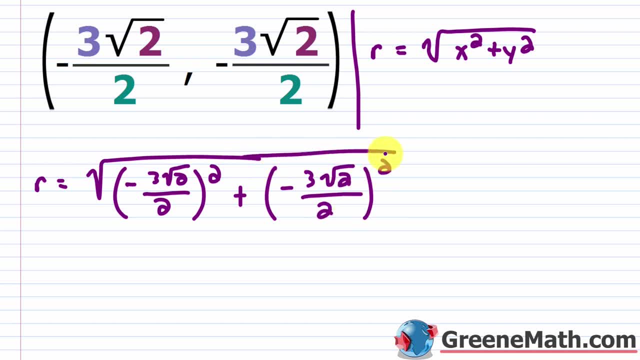 Let me make this a little bit longer, so it's proper. And so if I think about this, I know that negative in each case is going to be gone. right, Square root of negative, you get a positive. Three squared is nine. 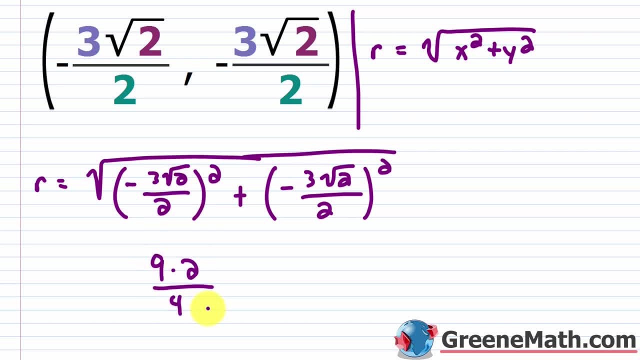 The square root of two squared is two, and then two squared is four. okay, So essentially, what I'm going to end up with is canceling this with this and getting a two. okay, So you'll end up with nine halves. So I'll have nine halves here and nine halves here. 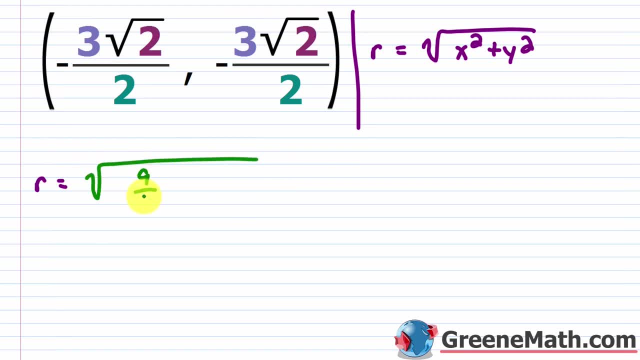 So basically I would have: r is equal to square root of nine halves plus nine halves. You have a common denominator there. So basically, nine plus nine is 18, you would have 18 divided by two, which is going to be nine. okay, 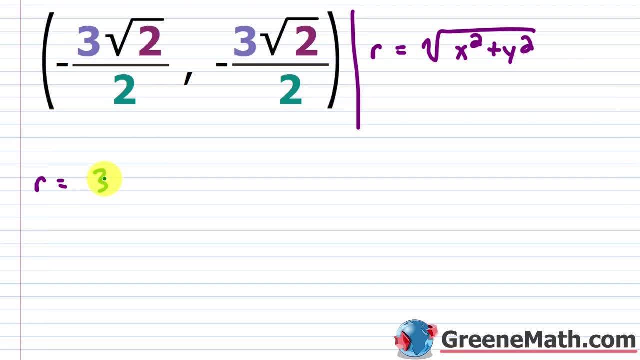 So r is equal to the square root of nine, which we know is three. okay, So let me erase this from over here. let me put this as: r is equal to three Now, when we think about the directed angle, theta, okay. 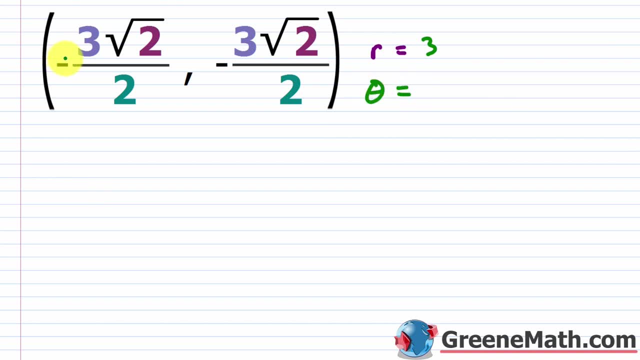 This is where it gets a little bit tricky. First off, consider that your x coordinate is negative and your y coordinate is negative. So if you think about this on your rectangular coordinate plane, if your x value is negative and your y value is negative, you're going to the left and you're going down. 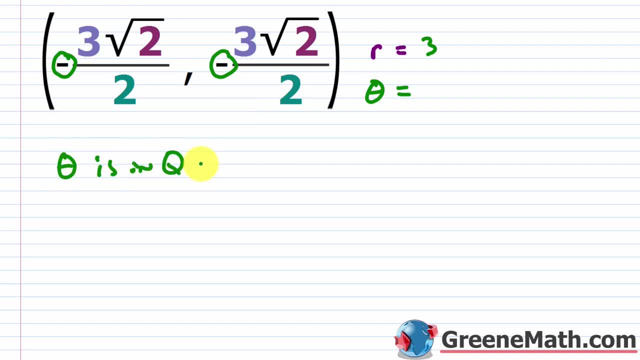 So that means that theta is in quadrant number three. okay, So let's keep that in mind. So let's do our inverse tangent function. If you have the same thing over itself, okay, and it's not zero, you're going to get one. 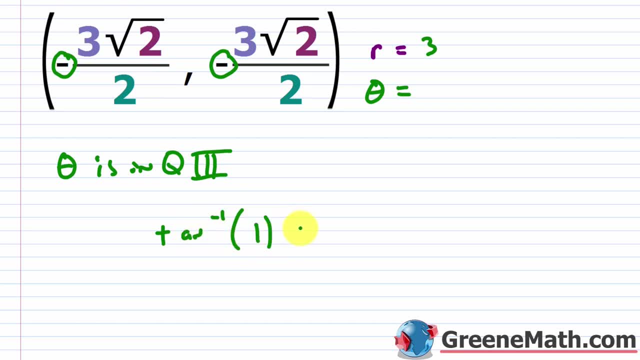 So, basically, I want this- The tangent inverse of one Type that into your calculator and you're going to get 45 degrees. So if I'm in quadrant three, what I want to do is I want to take 180 degrees and I want 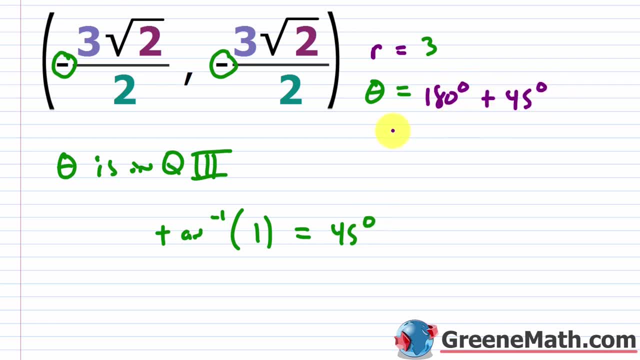 to add my reference angle there of 45 degrees and this is going to give me 225 degrees. Okay, so this is 225 degrees, So let's erase this. I'll just put that these are polar, so the polar coordinates. okay, like this would: 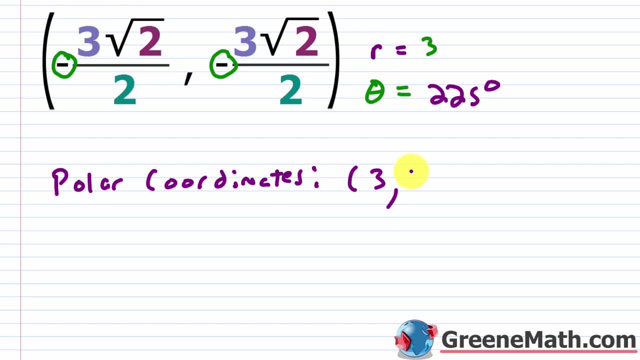 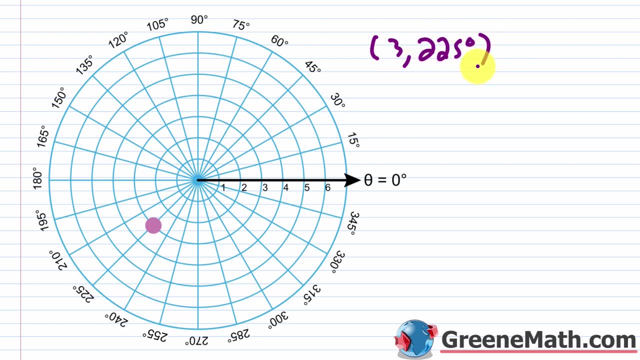 be, you would have three for your r value and then your theta value would be 225 degrees. So, to plot this guy, this is going to be 3, 225 degrees On our polar grid. basically, what we do to construct this grid. remember, you have your. 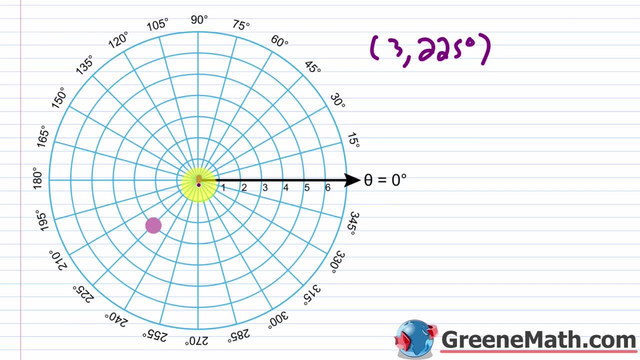 pole, or your origin. okay, let me make that visible- and essentially this is going to be the center for everything. okay, Then you're going to have your polar axis, which again is drawn in the direction of the positive x axis. So you have some notches here. 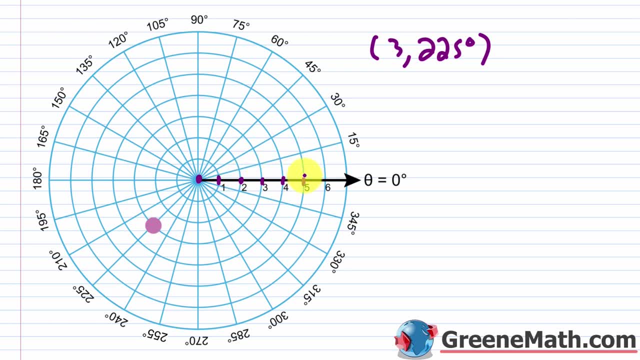 So this is 1, this is 2,, 3,, 4, you know so on and so forth, And basically what these are going to give you. you're going to make some circles and the first one is going to have a radius of 1, right. 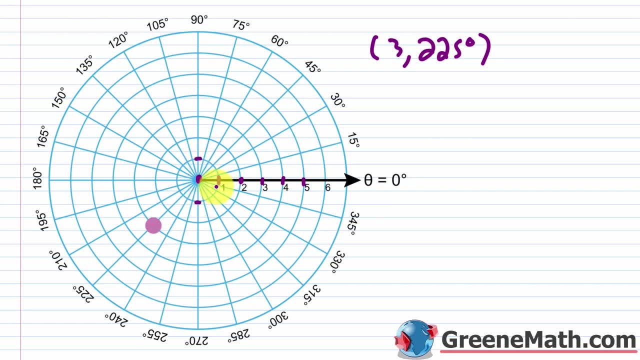 So basically up here, this is 1,. this would be negative 1 if you think about it as the regular Cartesian coordinate system, and this would be negative 1, right, But the distance from the center or the pole to any one of those points would be 1, right. 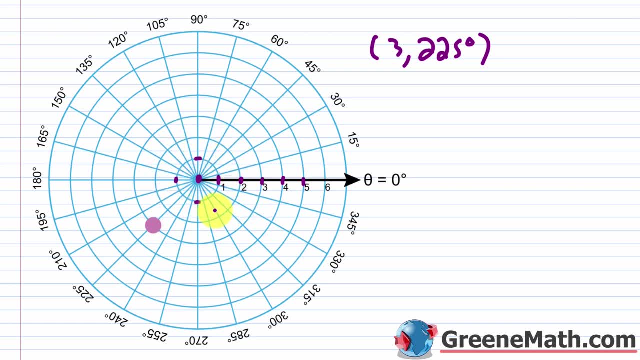 So that circle would have a radius of 1.. Then you have a circle with a radius of 2, then 3, then 4, then 5, you know so on and so forth. Then you also have these angles here which are in increments of 15 degrees, or if you're 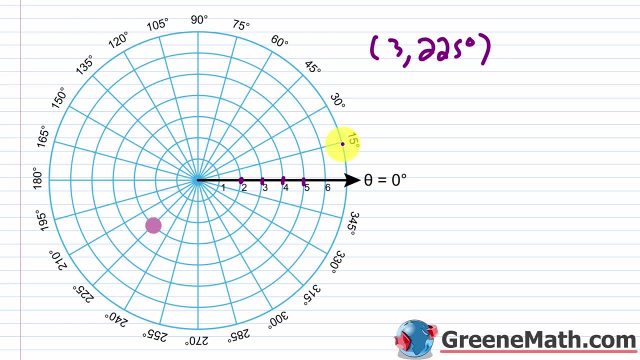 working with radians pi over 12 radians okay. So essentially, if I want this 3, 225 degrees, I'm finding the meeting point of a circle with a radius of 3, okay and an angle of 225 degrees. 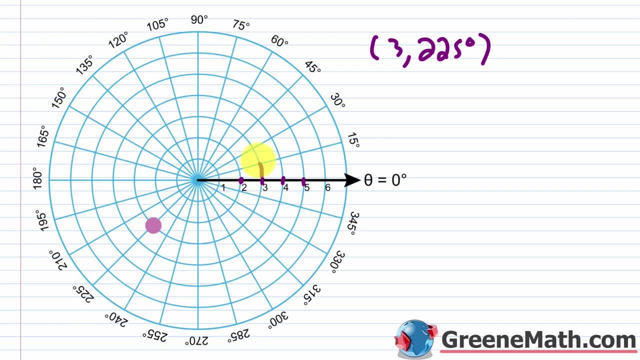 So I can come out to this circle with a radius of 3, and then I can swing around. okay, to this angle that's 225 degrees. So that's going to put me right here. Okay, So this would be the point on this polar grid where we have 3 as the radius and 225 degrees. 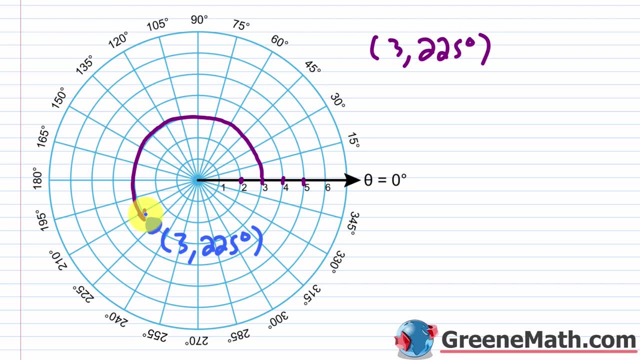 as the directed angle. okay, Now there's obviously other ways that you could name this point. I'm going to get to this later on. okay, You realize that you could swing around again 360 degrees, or you could actually rotate clockwise 360 degrees or multiples of that, okay. 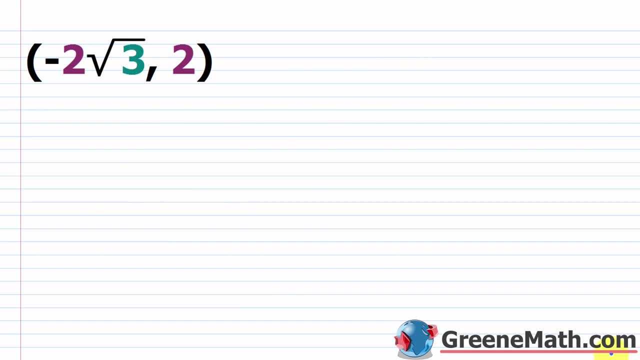 So we'll talk about that later on. All right, let's take a look at another example. So here we're, given the rectangular coordinates, We have the negative of 2 times square root of 3, comma 2.. So again, this is your x value and this is your y value. 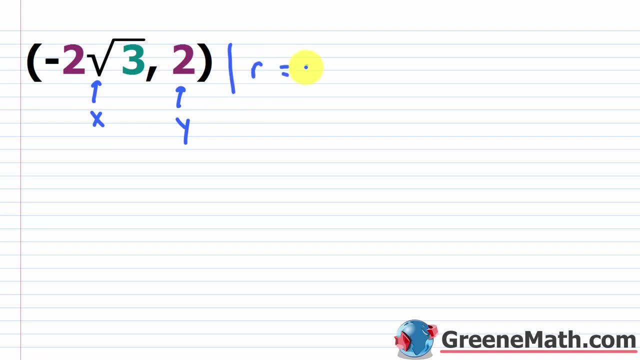 So to get the r value, what are we going to do? Remember, this is equal to the square root of. you take the x value squared, so the negative of 2 times square root of 3, okay, being squared, and then plus. you're going to go ahead and 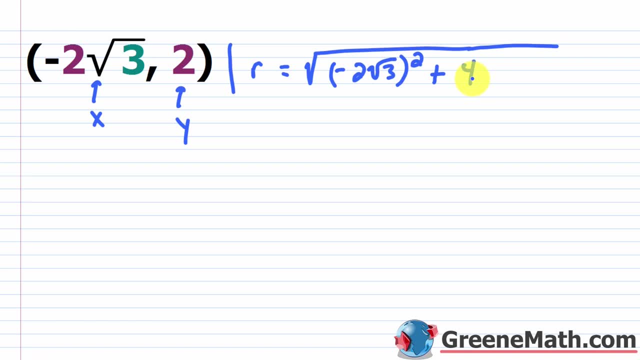 take the y value squared, So 2 squared. let's just go ahead and write 4, okay. So if I square negative 2, I get 4.. If I square the square root of 3, I get 4.. 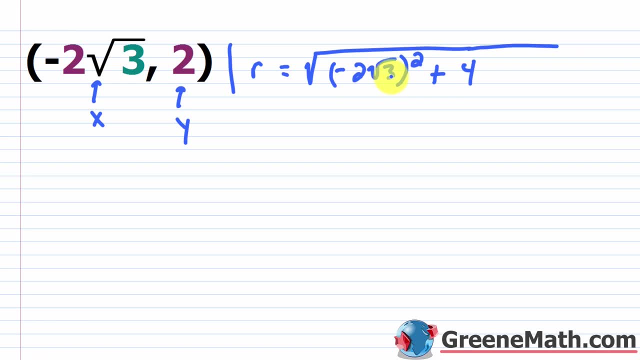 Okay, So this would be 4 times 3,, which is 12.. So let me go ahead and put a 12 in there, And 12 plus 4 is obviously 16, and the square root of 16 is going to be 4.. 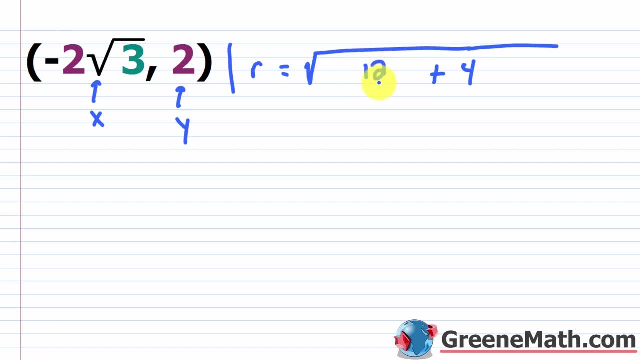 Okay, So we have the r value Again. that's pretty easy to get When you consider theta. okay, when you consider theta, you have to think about what quadrant you're in. So if my x value is negative and my y value is positive, that means I'm going to the left. 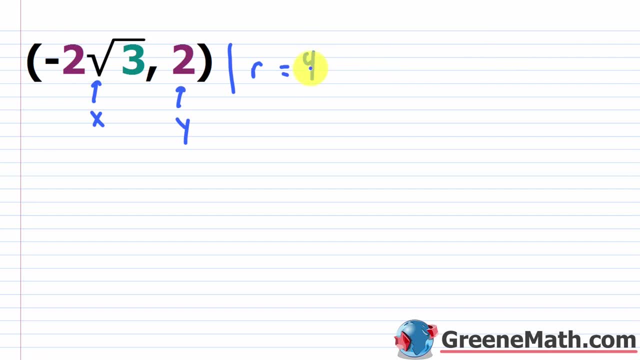 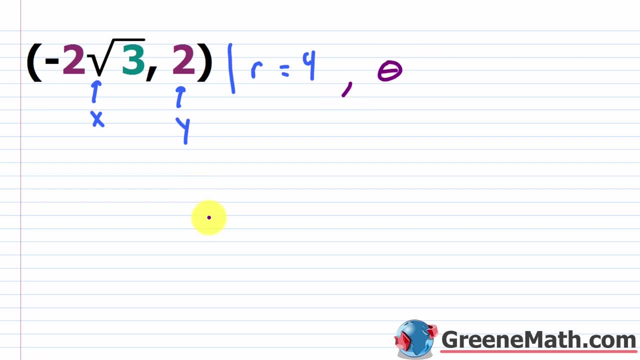 So I'm going to be in quadrant 2.. So I'm going to be in quadrant 2.. Okay, so always figure that out first. So theta is in quadrant 2. Okay, So theta is in quadrant 2. Okay. 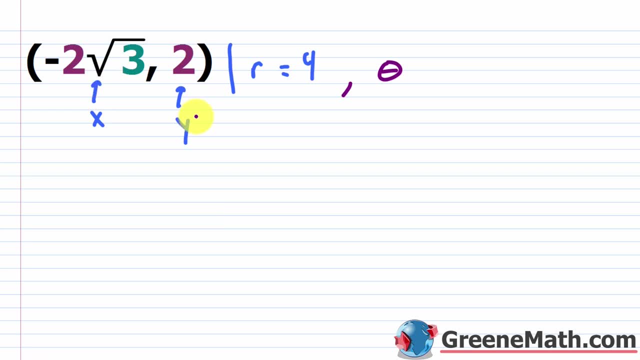 So always figure that out first. So, then, what I want to do is I want to think about: okay, well, the tangent of theta is equal to y, which is 2, over x, which is negative, 2, times the square root of 3.. 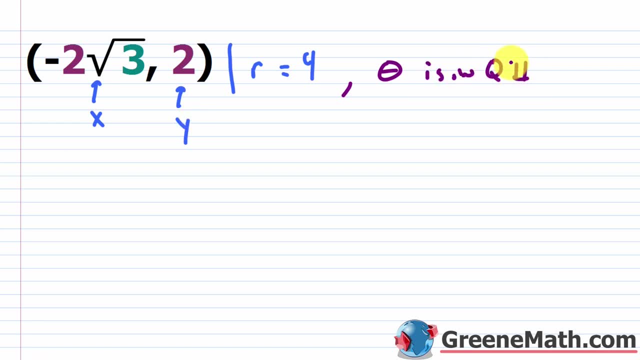 Let's go ahead and cancel this with this And basically I have 1 over theta minus once we finish the 1, that will give us 1 twice thex. All right, In that case, this earned us the кв 지금. 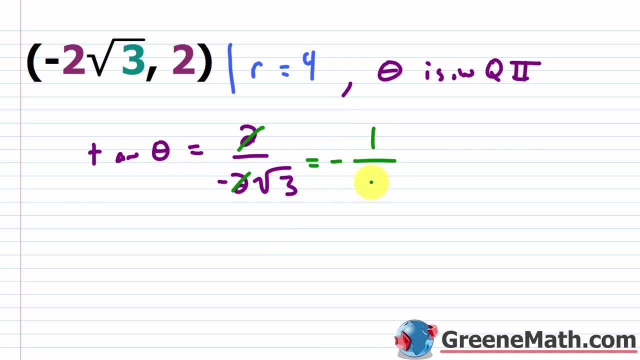 over, you would have the negative of the square root of 3.. Let's put the negative out in front and we'll put the square root of 3 over here, and then I'm going to rationalize the denominator. so square root of 3 over square root of 3.. So this becomes the negative of the square root of 3. 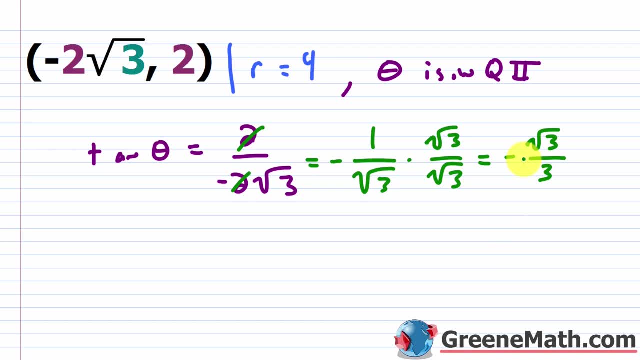 over 3.. Now I'm not going to use the negative, because I want something in quadrant 1 when I use my inverse tangent function. So let me erase all of this, okay? and basically what I'm going to do is I'm going to say I want the inverse tangent of. let me go ahead and make this positive, so I'll. 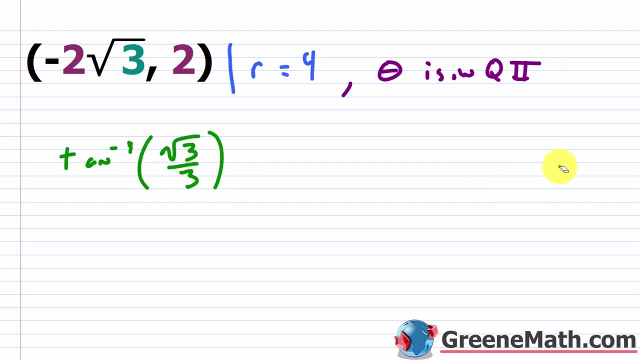 the square root of 3 over 3.. If I punch that into my calculator, I'm going to get 30 degrees. okay. so the way this works, if I'm in quadrant 2, okay, and I want an angle with a reference angle of 30 degrees, I want to take 180 degrees and subtract 30 degrees away from it. So basically my theta. 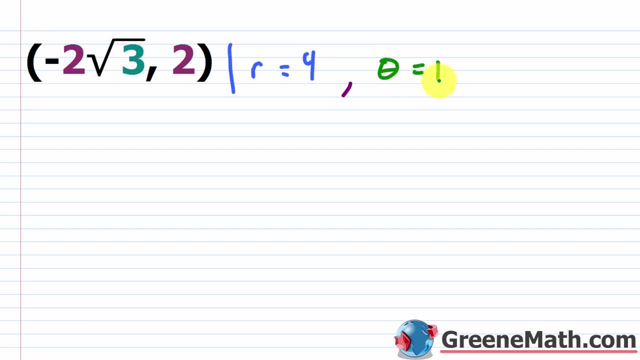 okay, my theta would be equal to 180 degrees minus 30 degrees, which is 150 degrees. okay, so 150 degrees, and I forgot to put my zero there, so let me put that in. so the polar coordinates are polar coordinates. let me write this out. the polar coordinates will be what it's: your r value comma, your theta value, so 4 comma. 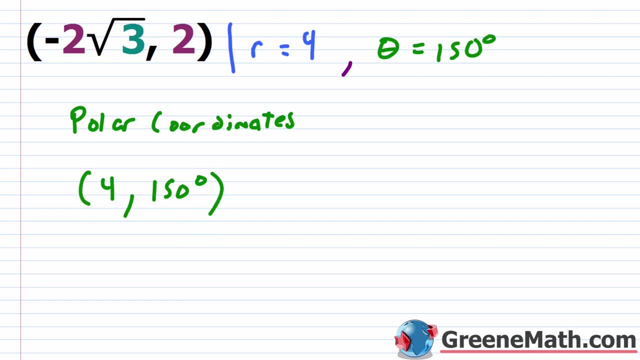 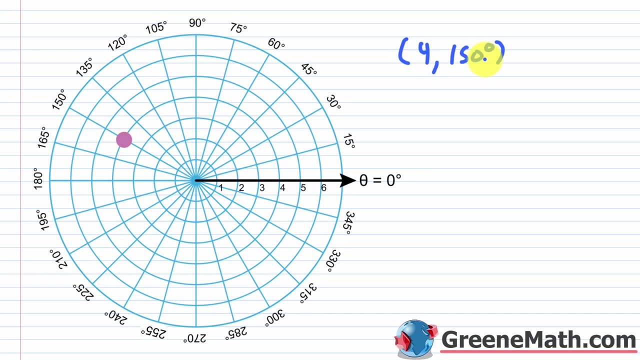 150 degrees. so to plot this so again the point would be 4 comma, 150 degrees as polar coordinates, and again all i'm going to do is i'm going to go out to a circle with a radius of 4, okay, and what i'm going to do from there is just swing around, okay, until i get to 150 degrees. let's go ahead. 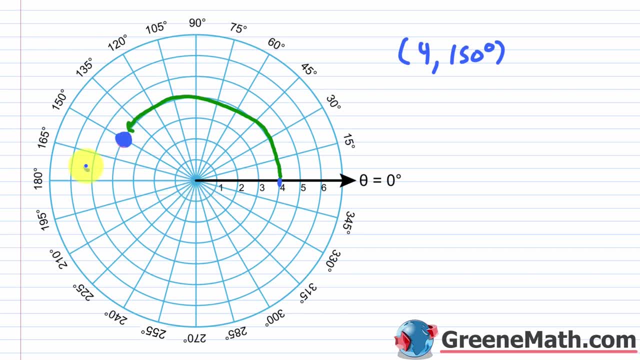 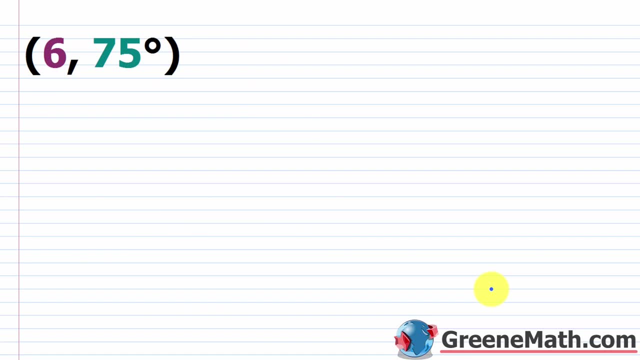 and plot that point right there. okay, so this is going to be 4 comma 150 degrees, again plotting this on the polar grid. all right, let's take a look at an example where we have polar coordinates and we want to convert to rectangular coordinates. so first off, we have 6 comma 75 degrees. let's just 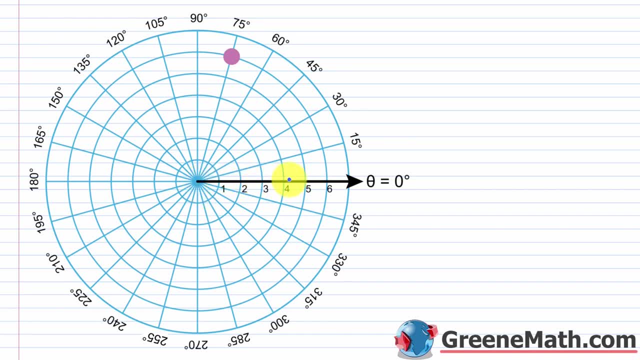 plot this real quick. so again, what i want to do. i want to go out to a circle with a radius of 6, okay so, right here, and then i'm going to swing around to an angle that's 75 degrees. that's going to put me right there. okay, so it's going to be my 0.6 comma, 75 degrees. all right, so. 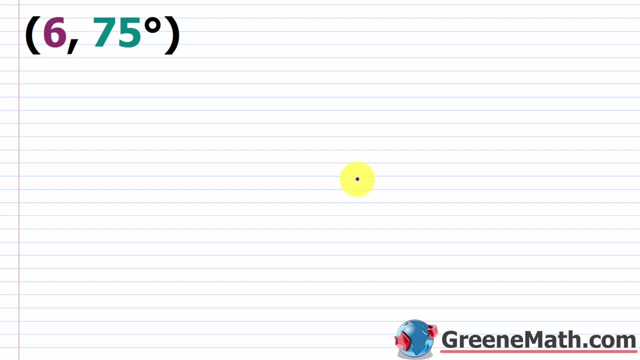 let's consider how to transform this into rectangular coordinates now. so remember, if we want to write this as x comma y, the relationship we talked about earlier is that x is equal to r times cosine of theta and that y is equal to r times the sine of theta. so these are two things. 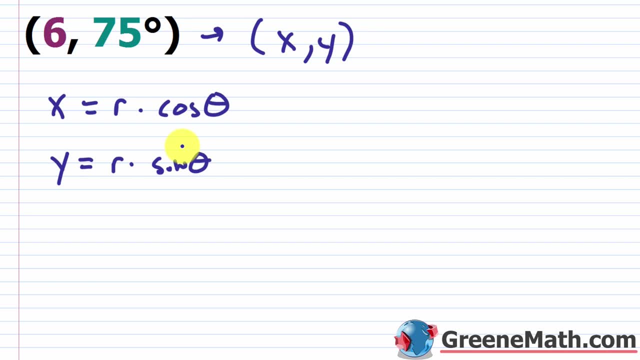 that we need to memorize. you're going to use it basically all the time. now, once we think about this, we have our r value of 6, so you might as well just put this as 6 in each case. okay, so 6 and then 6. 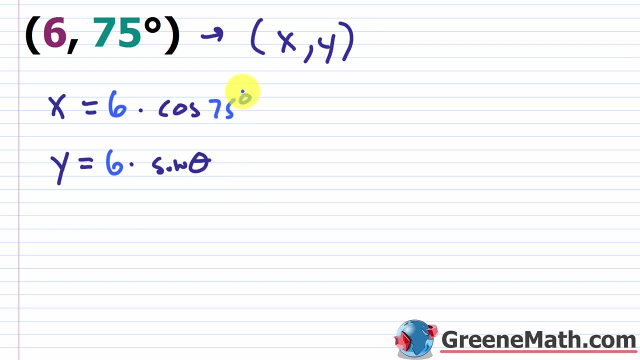 and then what is the cosine of 75 degrees and what is the sine of 75 degrees? so remember, this is not on your unit circle. okay, so what you can do is use identities- okay, we talked about this earlier in the course- to get an exact value. okay, if you punch it into your calculator, you get an approximation. 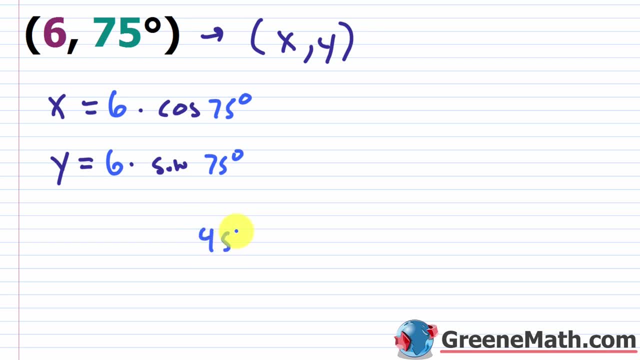 so you could write 75 degrees, 45 degrees plus 30 degrees, okay, and you could use your cosine sum identity or your sine sum identity, depending on what you're working with, to get the exact value. okay, i'm just going to give this to you because we don't want to spend time working on something we already did, so essentially. 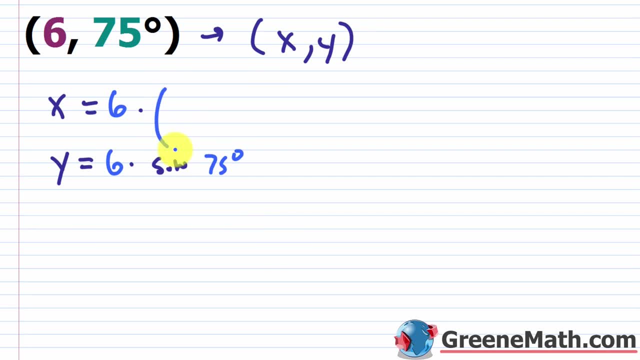 the cosine of 75 degrees. i'm going to put some parentheses here and i'll put it as the square to 6 minus the square to 2, and this is going to be over 4. okay, and then the sine of 75 degrees. again, i'm going to put- let me kind of slide this down a little bit here, so i'm going to put this: 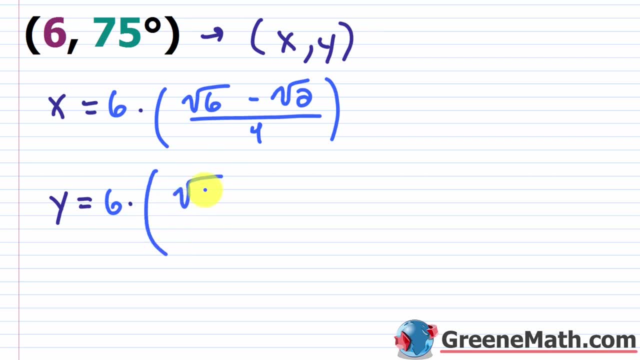 so it's not in the way i'm going to put this, as we'll have the square root of 6 plus the square root of 2, and this is going to be over 4. okay, so this is getting exact values, if you want to punch it. 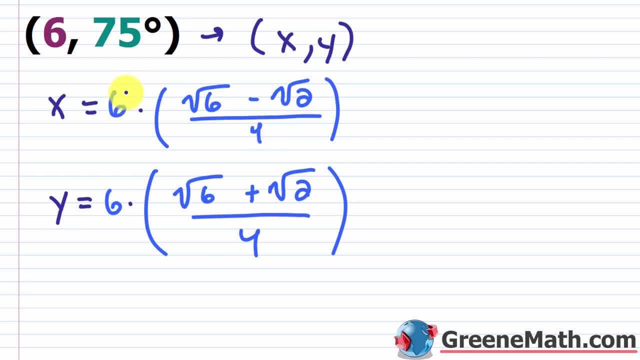 into your calculator approximated. you can do that too. it's up to you. so let's go ahead and cancel this with this. okay, so this would basically be a 3 and this would be a 2, okay, and then from there i would distribute this in, so i would have 3 times square root of 6. so 3 times square root of 6 minus. 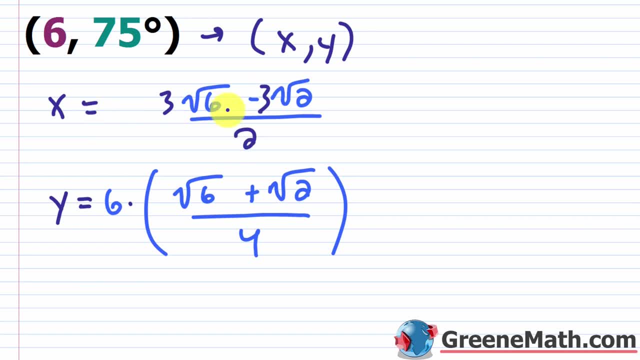 3 times square root of 2 and this is over 2. okay, so this is going to be your x squared. you don't get 2 squared by 2 if you are over 2.. coordinate then here. this cancels with this. again, this is the 3 and this is a 2, and then you're. 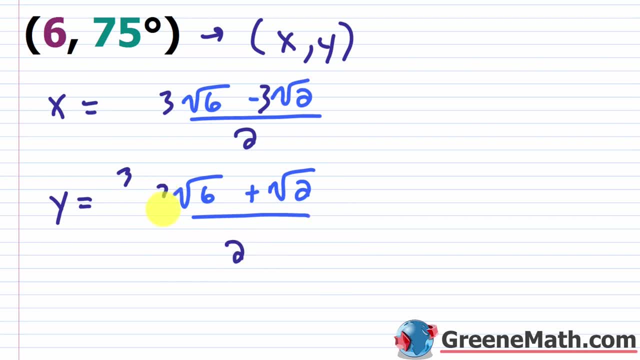 going to distribute that 3 into each, okay, so let me put this as a 2. this would be a 3 and this would be a 3. let me slide this down, so this would be 3 times square root of 2, okay, so if you want, 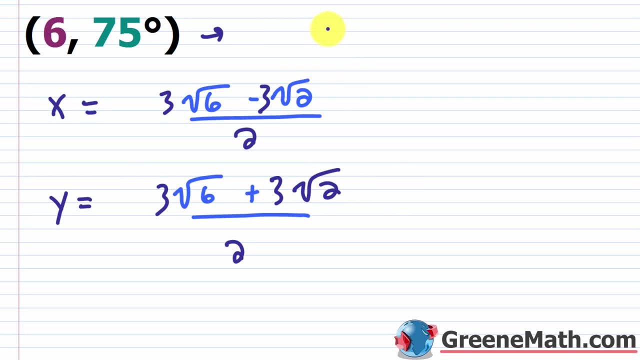 to write this as rectangular coordinates. you can go ahead and say that it would be 3 times square root of 6 minus 3 times square root of 2 over 2 and then comma. let me erase. this is all going to not fit, so let me slide this down a little bit so it all fits on the screen and then over here. 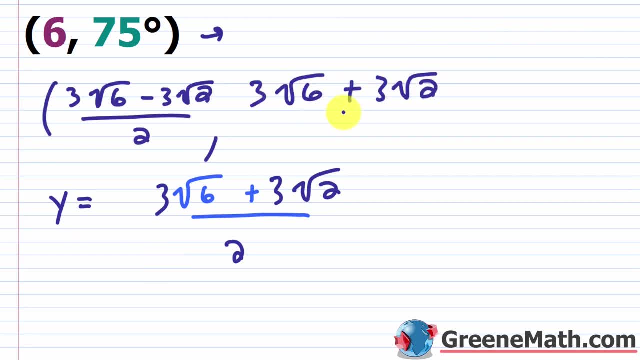 I have 3 times square root of 6 plus 3 times square root of 2 and then over 2. so kind of messy, kind of nasty. again, your teacher might allow you to approximate it, so it might be a little bit quicker for you to do it that way. all right, let's look at one more example where we're going from. 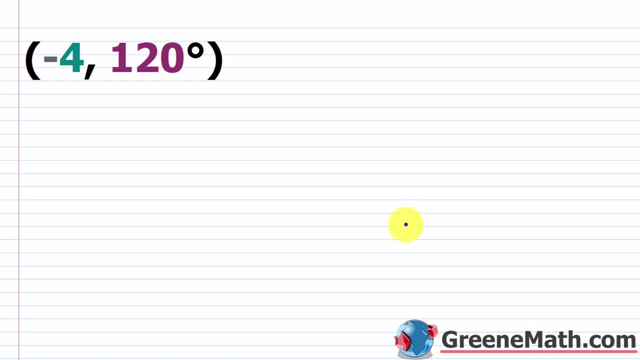 the polar coordinates to the rectangular coordinates. so here we have negative 4 comma 120 degrees. so the r value, okay, is going to be negative 4 and the theta is going to be 120 degrees. So let's pause for a minute. When you get an r value, that's negative. 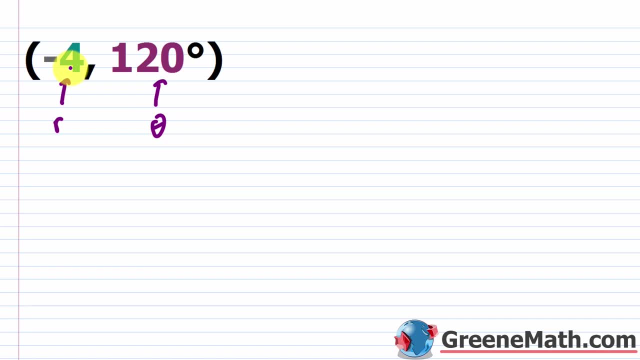 and you're asked to plot this guy. it can be a little bit confusing. okay, When you get a theta value, that's negative. that's pretty simple. We know that a negative angle just means I'm rotating clockwise right. So let's deal with this r value that's negative. first. Let's go to the polar grid. 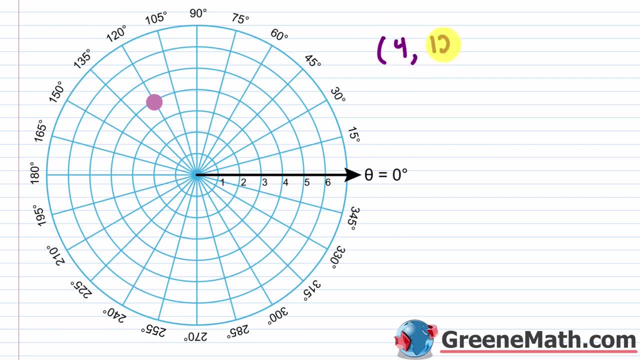 and let's first graph positive: 4 comma 120 degrees, and then we'll think about what negative 4 comma 120 degrees would mean, okay. So if I step out to a circle here with a radius of force, let me go out here, let me swing around, okay, And I'm just going to draw a little terminal ray. 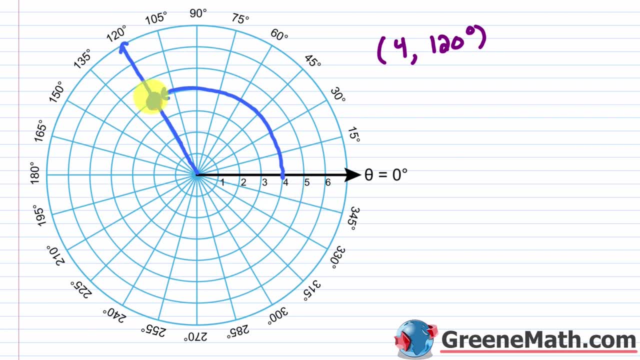 I'll do that the best that I can. I'm not a good drawer, But basically that point's going to be right there, okay, So you'll notice that that point is on that terminal ray. okay, So this is going to be the 4 comma, 120 degrees. okay, We know how to find that at this point. okay. Now, if I wanted to, 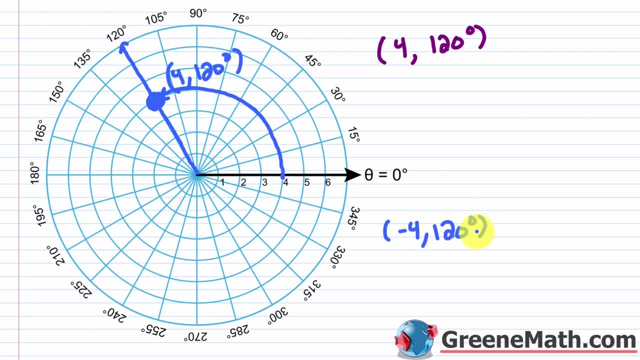 find negative 4 comma 120 degrees. I'm going to go out here and I'm going to draw a little terminal ray, okay, And I'm going to say negative 4 comma 120 degrees. All it means is that I'm basically 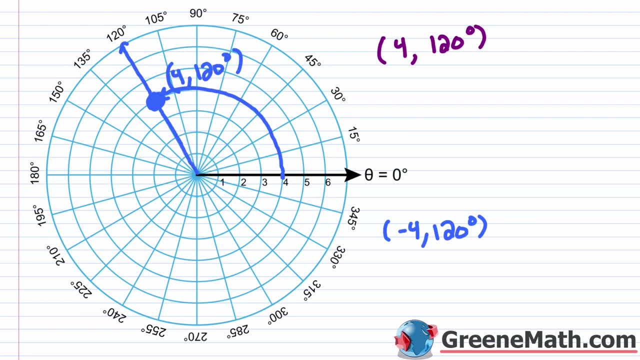 going to reflect this point across this pole, okay. So here's the pole, right here, and if I reflect it across the pole, I'm basically going to go in the opposite direction. So I'm going to go this way: 1,, 2,, 3,, 4 units. So that's going to be right there. okay, You can think about making a terminal. 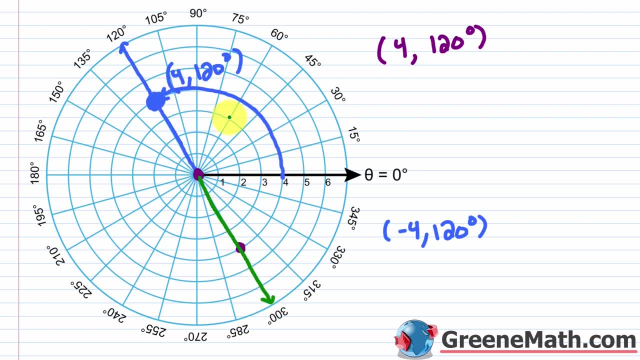 ray here and think about having the angle. let's say I had the angle, I could just start here and go all the way around. That would basically be a 300 degree angle. okay, so negative 4 comma 120 degrees would represent the same point has 4 comma 300 degrees. 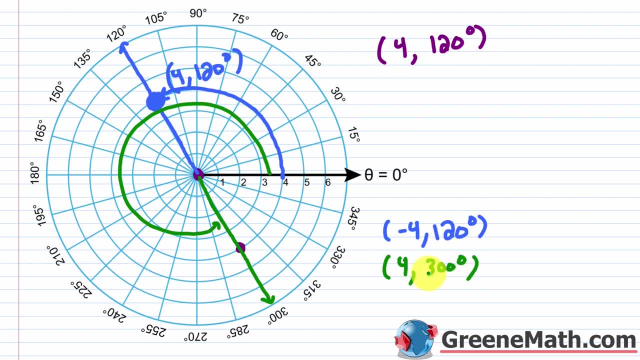 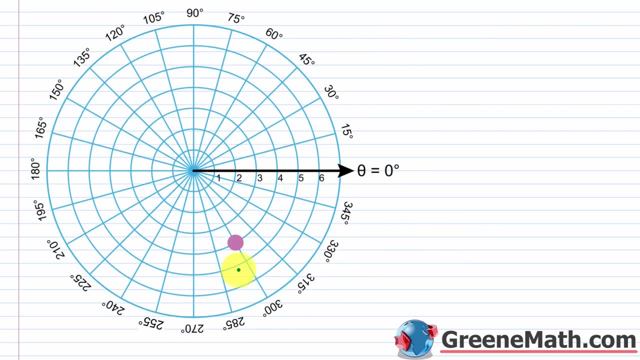 and we're going to talk more about these different forms in a moment. okay, but for right now, you could see a few different ways that you could go about finding this. so let me go to a fresh sheet here where this is already plotted. so the first thing, i'm going to label this as negative 4 comma. i'm 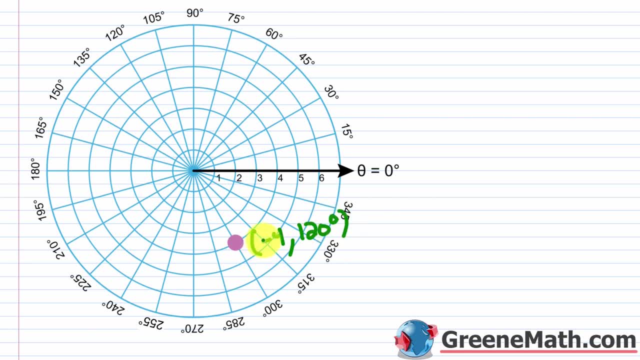 going to do 120 degrees. okay, i could have found this by going to 120 degrees like this, and then basically, just instead of going forwards, i would just go backwards by 4 units. okay, that's probably the easiest explanation, so i would just say: okay, i'm here, so i'm going to go 1, i'm going to go 2. 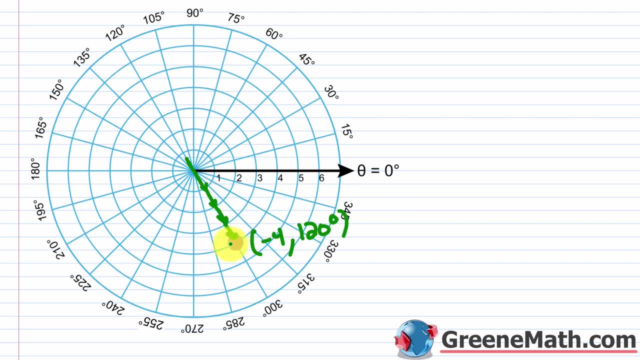 i'm going to go 3, i'm going to go 4, so out to a circle that has a radius of 4, right, i'm just turning around and going backwards. that's what the negative 4 is basically telling you. okay, so that would be one way i could get to my point. another way, and this might be helpful for you: 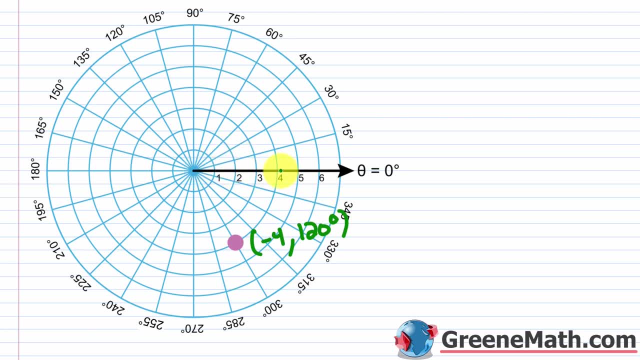 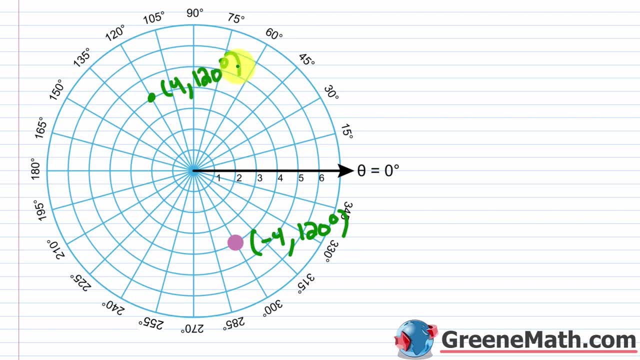 be right there. so this is my 4 comma: 120 degrees. and notice that if i wanted to swing over here, okay, i'm basically going to add 180 degrees to this angle. okay, or i could subtract 180 degrees from the angle as well if i wanted to. so i could either say that this is going to be plus 180. 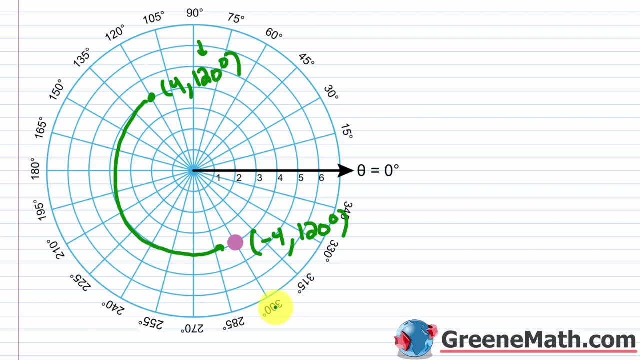 degrees, which would be 300 degrees. or i could subtract away 180 degrees and say this is negative 60 degrees. if i wanted to rotate clockwise, okay, but essentially those are the ways that you could think about doing this. once you graph these a few times, it becomes a little bit easier to work with in your mind. but just know if you 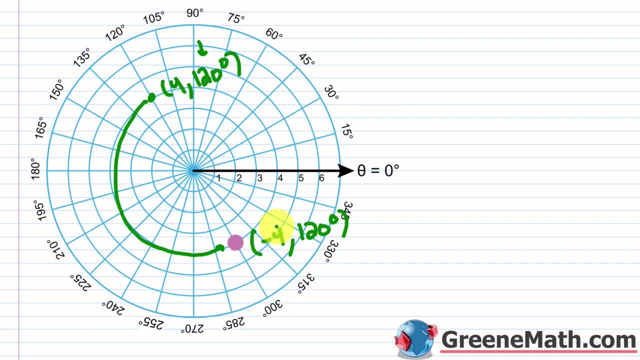 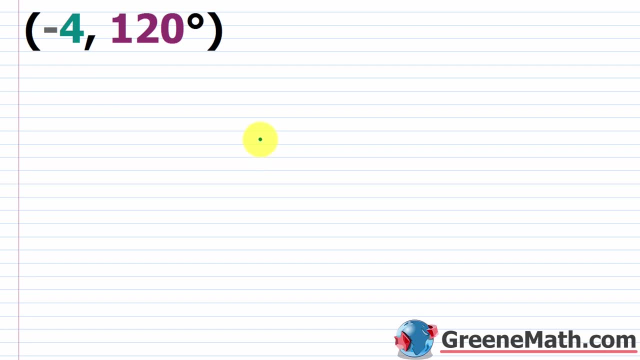 have a negative r value. you're basically going to walk backwards. okay, that's what it means. so let's go back and let's think about putting this into rectangular form. okay, so we know again that our x value is equal to. we would have the r value, which is negative 4 times the cosine of 120 degrees. 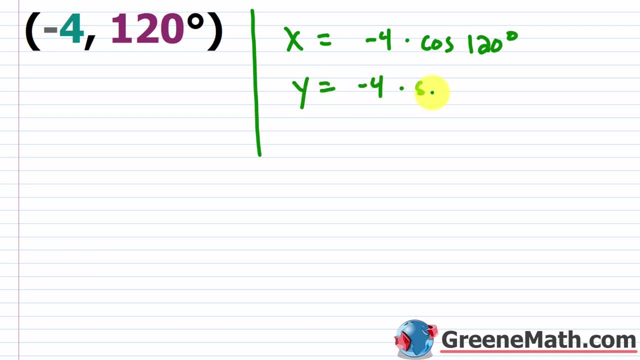 and the y value is negative 4 times the sine of 120 degrees. okay, so we know that 120 degrees is going to be. in quadrant 2. it's got a 60 degree reference angle and the cosine of 60 degrees is going to be a half. okay, but cosine is negative, okay, in quadrant. 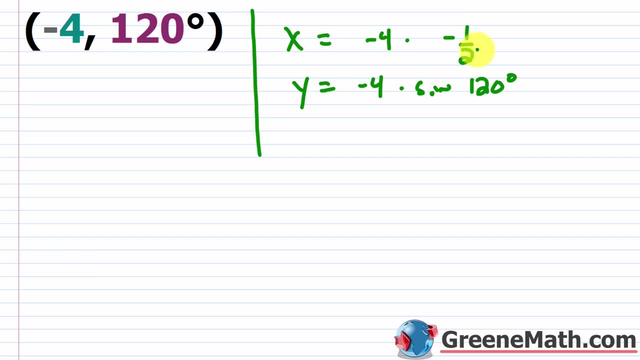 2. so this would be negative one half. so times negative one half. so of course this would be positive 2. so the x value is positive 2. very easy to find: the sine of 120 degrees. again, a 60 degree reference angle sine is positive in quadrant 2. so the sine of 60 degrees is square root of 3 over 2. 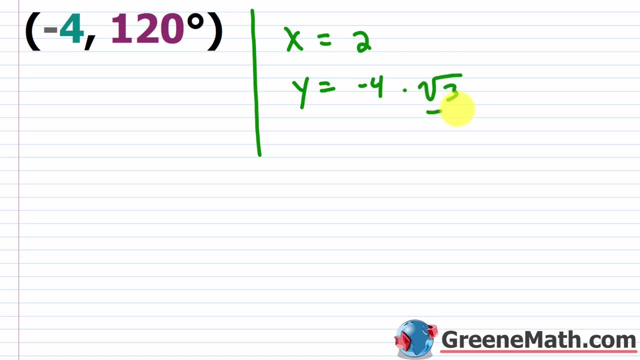 so this is going to be times the square root of 3 over 2. i can cancel this with this and i would have the negative of 2 times square root of 3, so negative 2 times square root of 3. so then my rectangular coordinates would be 2 comma. negative 2 times square root of 3. okay, so basically i want. 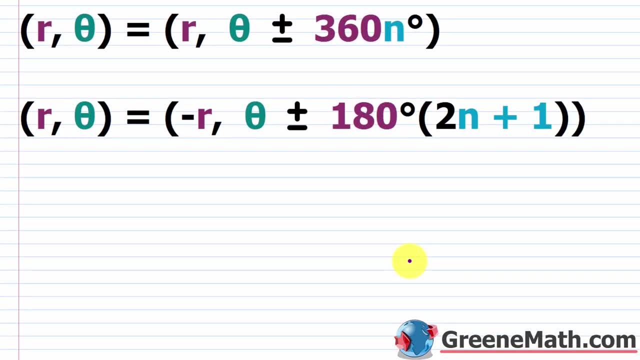 to go from here into our next point, which is talking about alternative forms for coordinates of a point in polar form. so for a given point in the rectangular coordinate plane you're going to have an infinite number of pairs of polar coordinates. so sometimes your teacher will say: 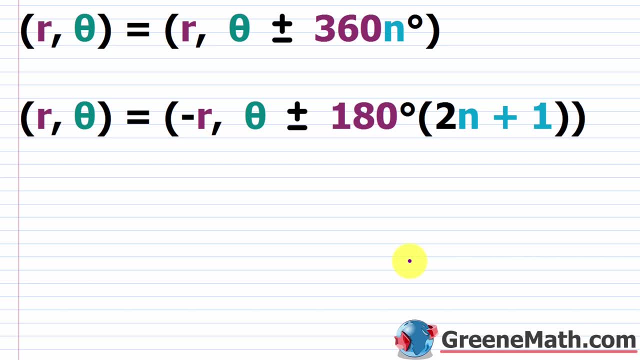 give me, you know, four examples of other polar coordinates that are the same as this polar coordinate i'm giving you. sometimes they want a general formula, so i'm just going to give you the general formula here and then you can apply that based on the example you get. okay, so the 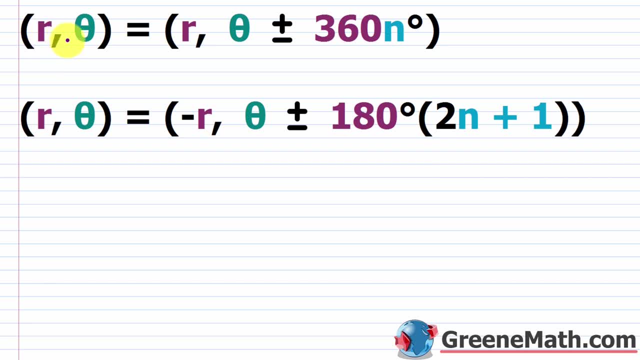 first one is pretty easy to understand. if we have some r comma theta, this is the same as if i said r comma and then you're a theta plus 360 times n degrees and just any integer or theta minus 360 times n degrees. now the plus or minus here is given in. 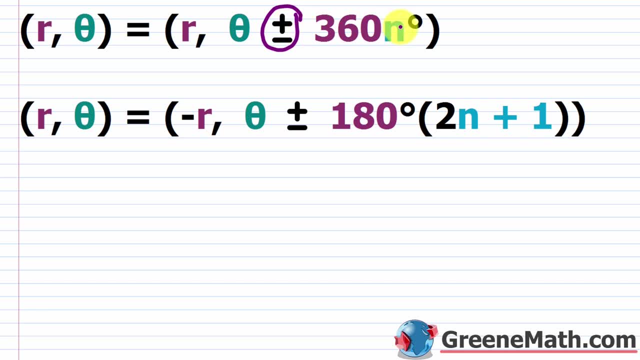 some books you really don't need it. you could just put plus because n is any integer. so you can make a positive, you can make it negative, you can do whatever you want. okay, but some books will put plus or minus, others will just put plus. if you go back to, let's say, this guy right here, where we 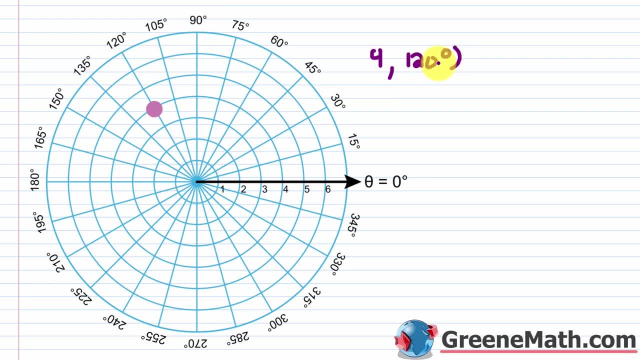 have 4 comma, 120 degrees. well, if you think about it, i could add 360 degrees to this and i could say: well, also, the same point could be located if i said 4 comma, this would be 480 degrees. right, because basically from here i would swing around. 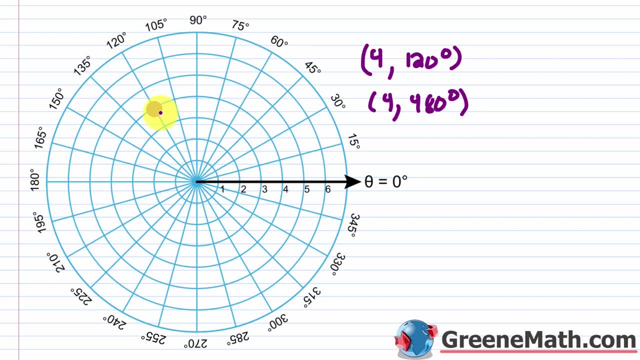 another 360 degrees and be right back to that same point. i could add 360 degrees again and get to 840 degrees. then i could do it again, and, again, and again. and the same thing is true if i subtracted 360 degrees away from 120 degrees. so some other coordinates would be something like: 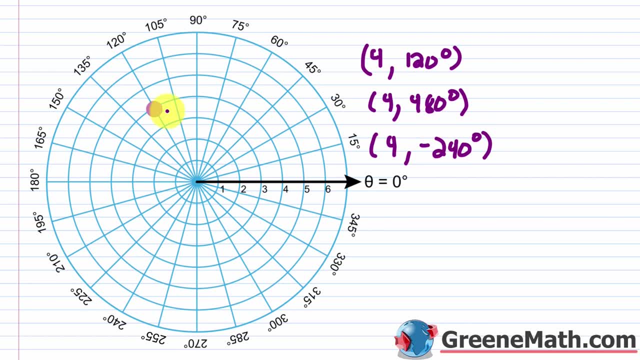 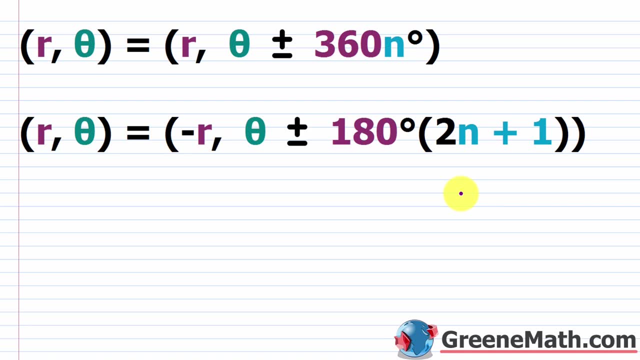 4 comma, negative 240 degrees. okay, so that would all locate the same point, okay. so now let's look at this second formula. this one is a little bit more difficult to understand because it's a little challenging to understand. but remember, if you have r and you have the negative of r, remember when. 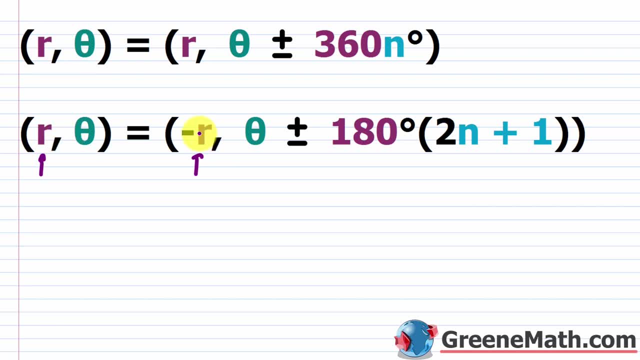 you think about the negative of r, you're basically going to be walking backwards. okay, so this is what this is related to. so again, you have this theta. whatever your angle is plus or minus, you're going to have this 180 degrees times this quantity. so let me distribute this out, so i'm going to put 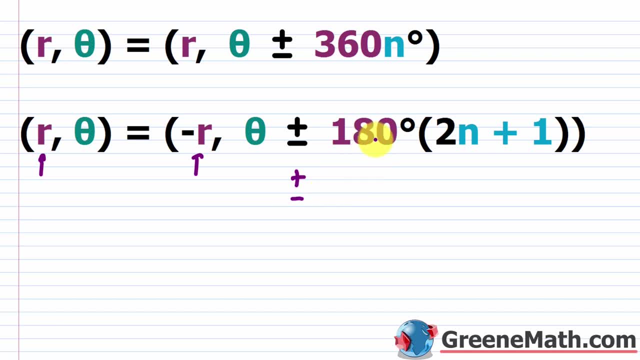 plus or minus, and i'll go ahead and say: you'll have your 180 degrees times 2n, so let's say this. and then i'll say plus. i'll go ahead and say: do my 180 degrees like this? okay, so you can have positive or you can have negative. you're going to see that you can actually drop the plus or minus. 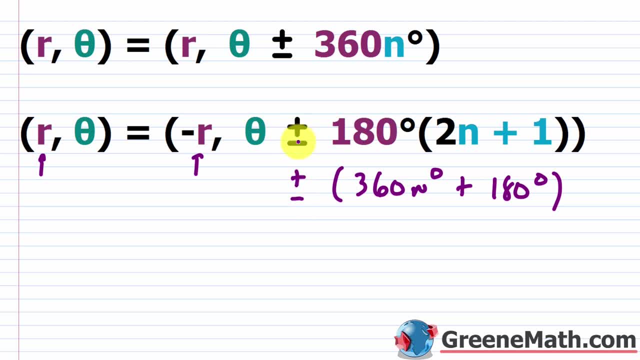 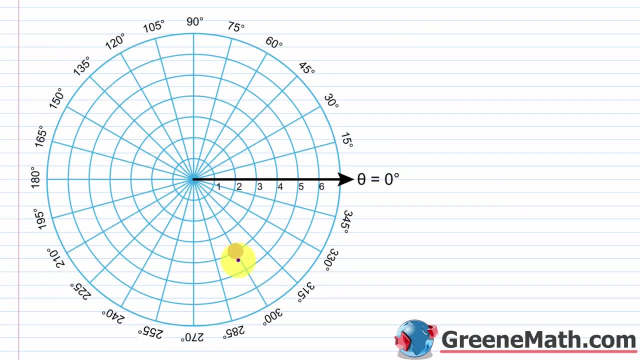 here as well. i'll go through some examples and prove that to you. most books will just write this with a plus sign, but others put plus or minus. okay, so it's, it's right either way. so if we go back and we think about alternative ways to locate this point, remember this was negative 4 comma 120. 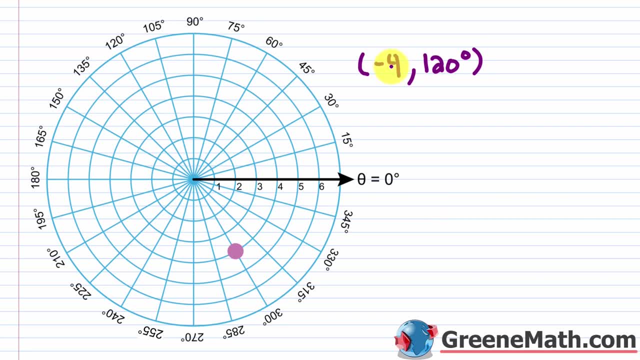 degrees, okay. so all we're saying is that we could have done the negative- 4 comma, 120 degrees- and then negative of this number, so that's 4 comma, and then i could add or subtract 180 degrees to this. so if i add 180 degrees i would be at 300 degrees. okay, so in other words, i could have gone out to: 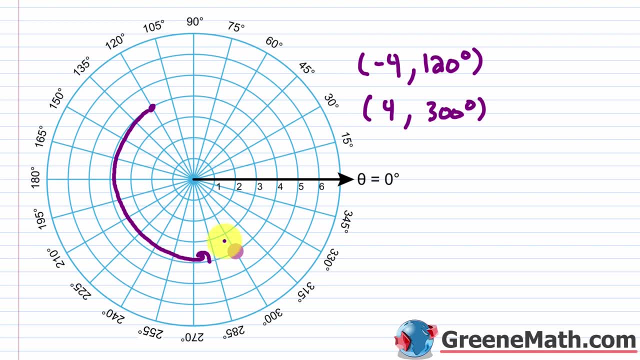 right here, and then i could have swung by 180 degrees this way right to get to 4 comma, 300 degrees. or i could have started there and i could have swung 180 degrees. this way. this would be clockwise, so that would be me subtracting 180 degrees, so i could have also said: this is 4 comma. 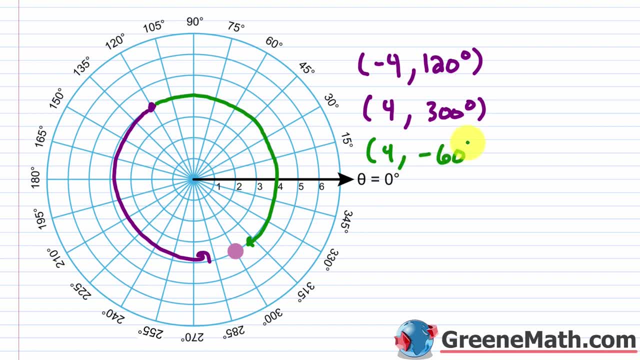 if i subtract 180 degrees from this, i would get negative 60 degrees. now, once i've added or subtracted the 180 degrees, i could then swing by multiples of 360 degrees. right, either positive or negative. so that's where these formulas are coming from, because from here i could say: okay, well, this is 4 comma 300 degrees. 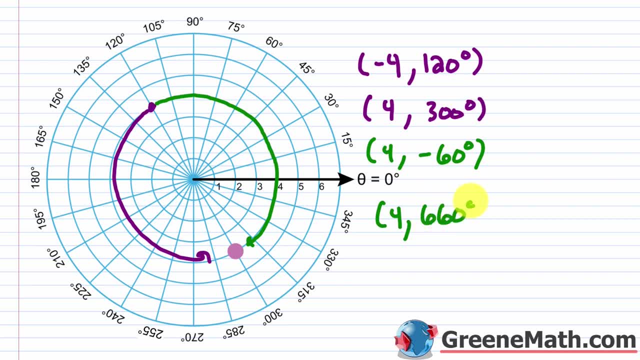 plus 360 degrees would be 660 degrees, okay, so that's another way to locate that point. so, in other words, i could have started here and i could have swung around 180 degrees, okay, and swung around 180 degrees and then swung around 180 degrees, and then swung around 180 degrees, and 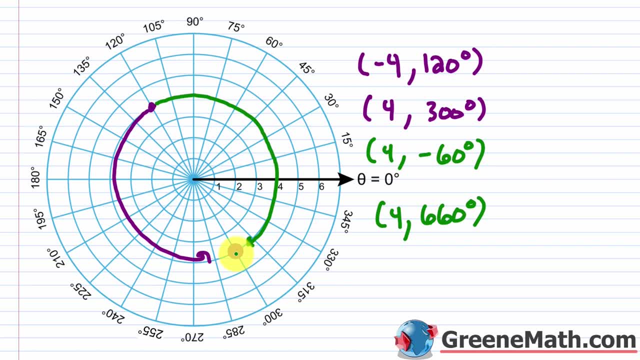 then swung around another 360 degrees to get to that same point. okay, also what i could have done: i could have started at 4 comma, negative 60, and i could subtract away another 360 degrees, which would be negative 420 degrees again- another way to locate the same point. so there's a lot of. 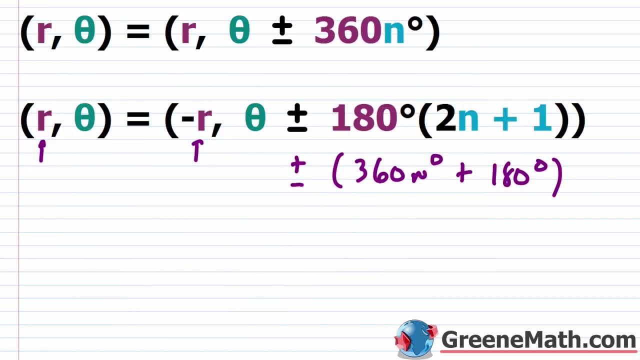 different ways you could have done this. so again, we put this into this nice little convenient formula, okay? so basically, it relies on the fact that you're first adding 180 degrees and then from there you could add 360 degrees, and then you could add another 360 degrees and then you could add another. 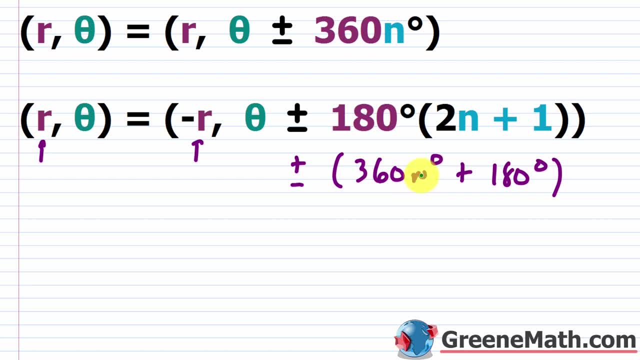 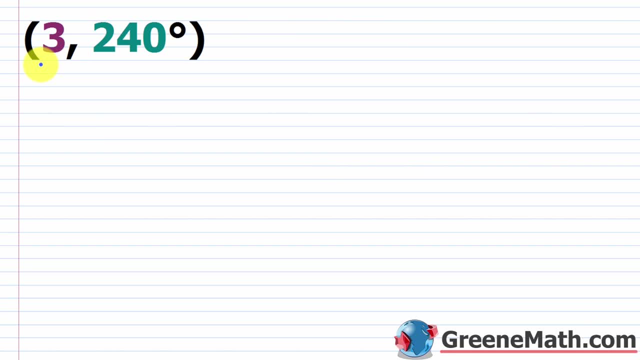 WAS, and then you could add- you could addARY degrees in there if you wanted to. so i think i'm thinking about it with a alternative in that, if you get the blasting you have started here, it's actually incredibly easy and you can start with three different ways. pierce right, except if 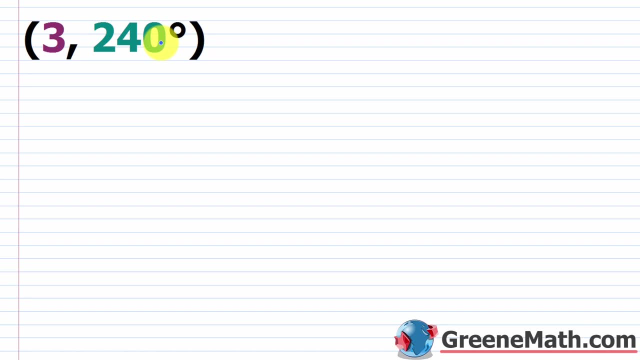 you want to do the polar coordinates 곳 and the polar coordinates of start by saying okay, the three would be the same, And what I would do here is I would add 360 times n to this right. So the formula you saw was theta plus or minus 360, and you would do. 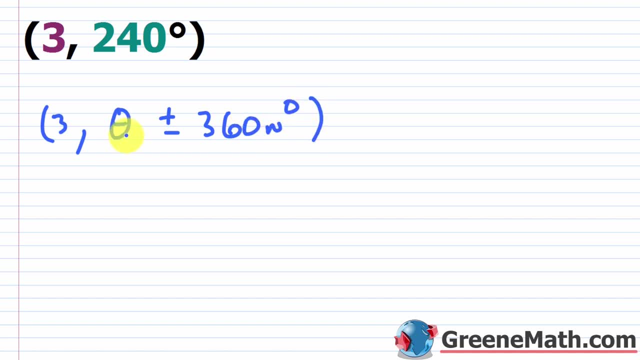 n degrees. okay, like this: Well, theta is 240 degrees, So let me put that in there. So 240 degrees and then plus or minus your 360 times n. Well, I don't need the plus or minus, because I can. 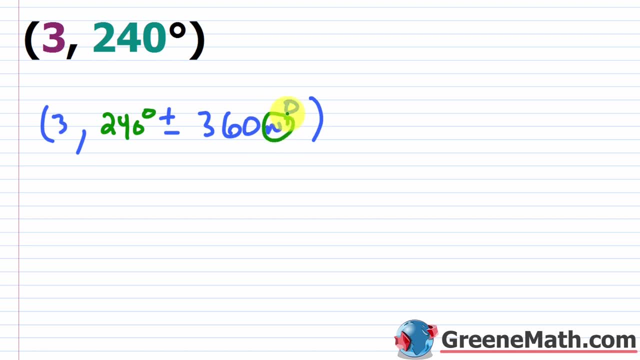 get anywhere. I want to go by just varying n right, n is any integer, so it could be positive, it could be negative. So again, you can put plus or minus. it's not wrong. but really most books will just put plus. You don't need the minus, So let's go ahead and get rid of it, Okay. 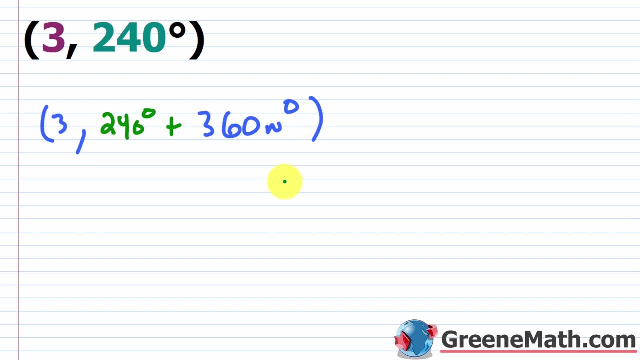 so the next one is a little bit more challenging to understand. So remember you would put the negative of whatever this number is. So in this case it's three. So I'm going to go ahead and put negative three and then I'm going to put a comma And let me go through and work out the 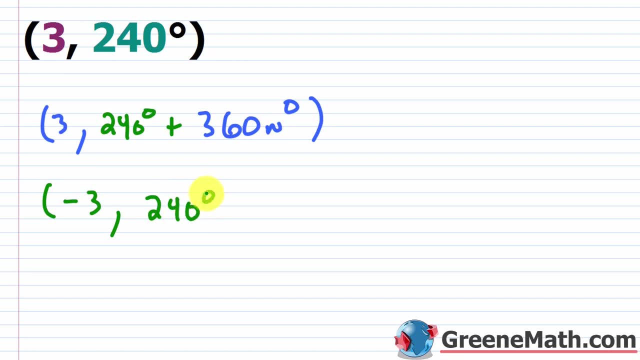 two different scenarios. So I'm going to go ahead and say: I have 240 degrees, okay. then I'm going to go plus- remember, you're going to have your 180 degrees and then you're going to have plus your 360, okay, n degrees. So this is basically where I'm swinging 180 degrees And then from 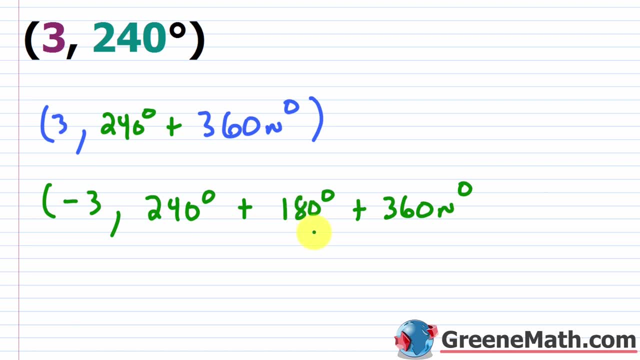 there I can add multiples of 360 degrees. I'm also going to do this with the minus sign to show you it comes out the same. So let me close this real quick negative three comma. I would do 240 degrees and then minus 180 degrees and then minus 360 n degrees. Okay, So basically. 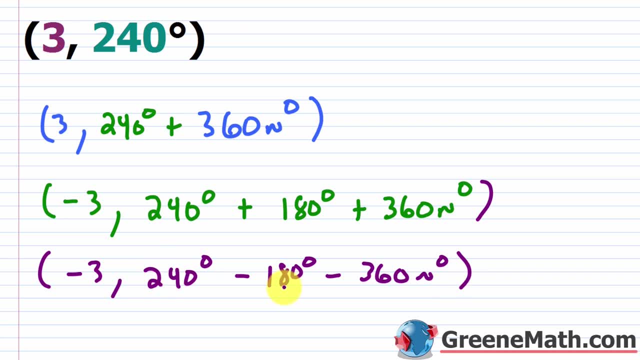 for this one: 240 degrees minus 180 degrees would be 60 degrees. Okay, so this would be 60 degrees. And then let me just tighten this down a little bit. we're going to end up erasing this one, So it doesn't really matter. Then this one, 240 degrees plus 180 degrees, is 420 degrees, Okay. 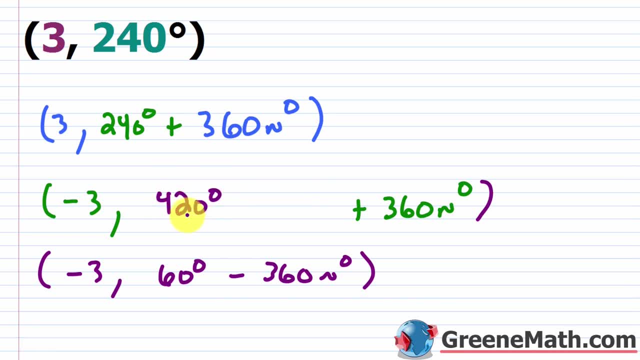 so 420 degrees And if you think about it, 420 degrees if I subtract off 360 degrees, this is going to be co terminal with 60 degrees. So really I could just put this as 60 degrees, okay, And this: 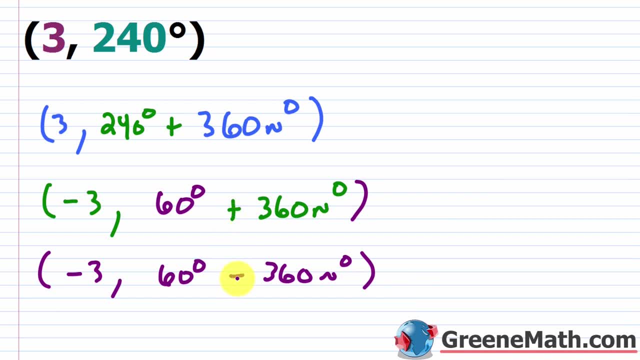 is going to give me the plus sign. So I'm going to put this as 60 degrees. So I'm going to put this down. And now we want to think about this: Do I need the plus or minus here? No, because I can. 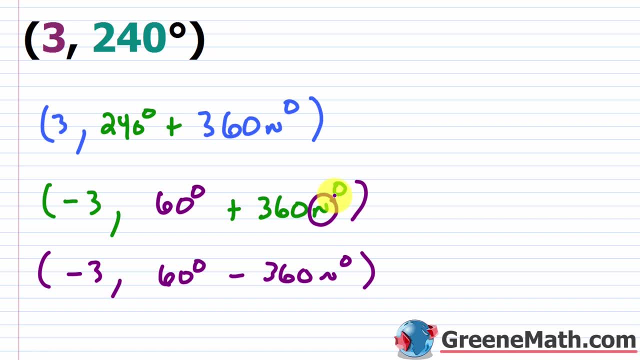 get wherever I want to go by just plugging in different integers for n right. If I want to do negative, I want to do positive, I'm allowed to plug in whatever I want there as long as it's integer. So I can go ahead and get rid of this, okay, and just list it with the plus sign Again. 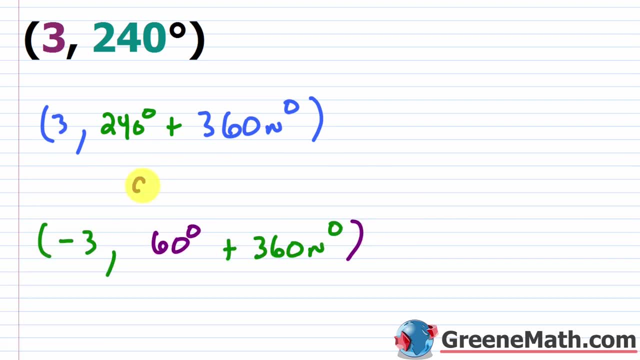 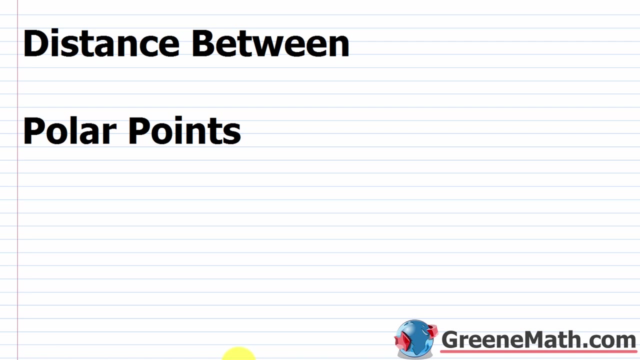 if you want to put plus or minus, it's not wrong, but it's just overkill, right? So I'm going to list this as my answer. So three comma 240 degrees plus 360 n degrees and negative three comma 60 degrees plus 360 n degrees. In this lesson we want to find the distance between polar points. 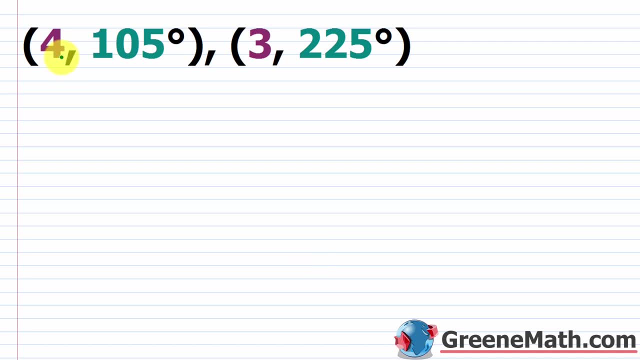 All right. so let's say that I asked you to find the distance between this four comma 105 degrees and three comma 225 degrees. How could we do this? We know that if we have the rectangular coordinates right and we're working on the rectangular coordinate plane, we can just use 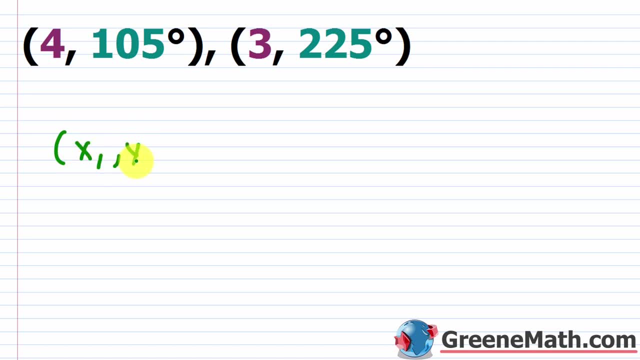 our distance formula right. So if I have two points, let's say x sub one comma, y sub one, Again, it doesn't matter which point you label as which I can plug into my distance formula. Let's say d, the distance between the two points is the square root of. I'm going to say x sub two. 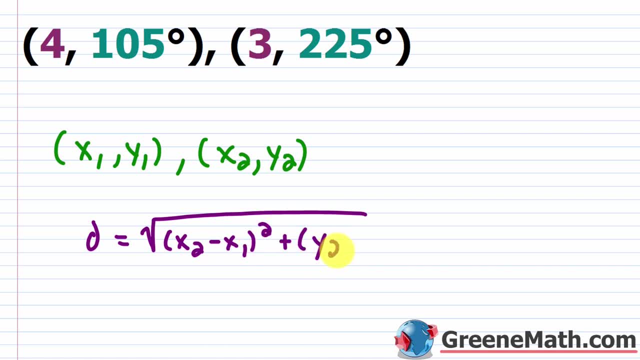 minus x sub one quantity squared. plus we have this y sub two minus y sub one quantity squared. okay, So this works for rectangular coordinates, but I have polar coordinates. okay, So what you could do- and I don't advise you to do this- you could go: x is equal to r times. cosine of theta. 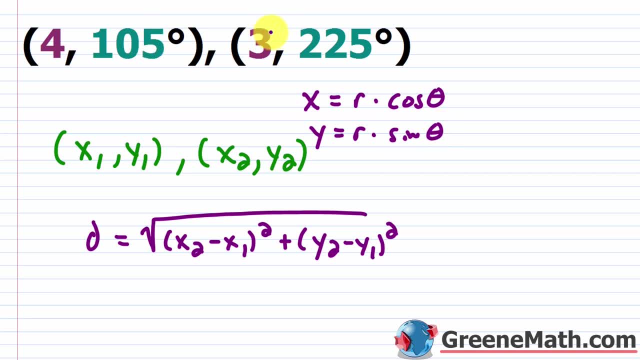 and y is equal to r times the sine of theta, So you could use that to convert these guys over. okay, Then you could plug in and you'd have your answer. But there's an easier way. okay, We can derive ourselves a little distance formula when we have these polar coordinates, So we could plug. 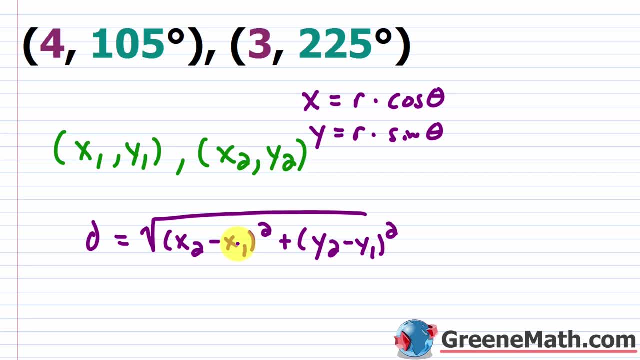 into this generically, change up a little bit of notation and come up with a formula. that way I'll do that at the end of the lesson, because I think it's a bit boring. I want to show you this using the law of cosines. I think it's a little bit easier to follow, okay, So let me erase. 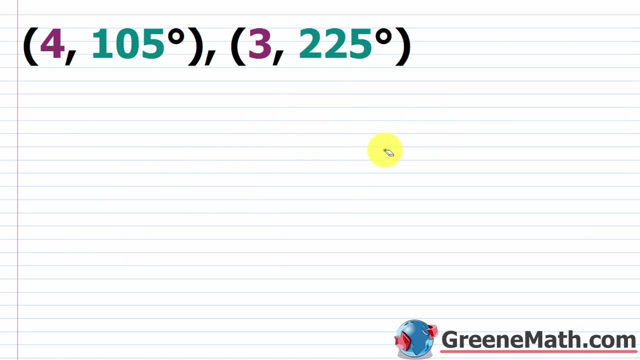 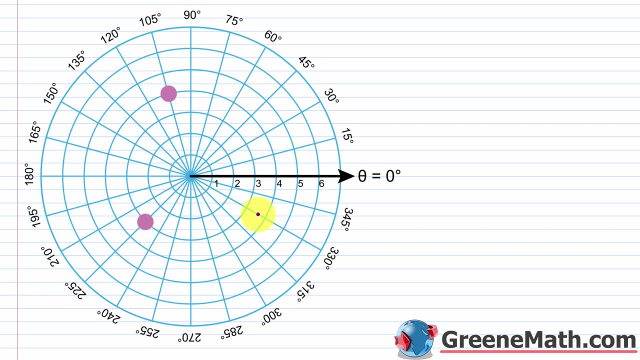 this real quick and erase this. And let's just start by plotting these two on the polar grid. okay, So we'll come down here and first I'll plot this 4 comma: 105 degrees. So you're going to step out 1,, 2,, 3,, 4 units. okay, So we're going to swing around to 105 degrees. So this is 4 comma. 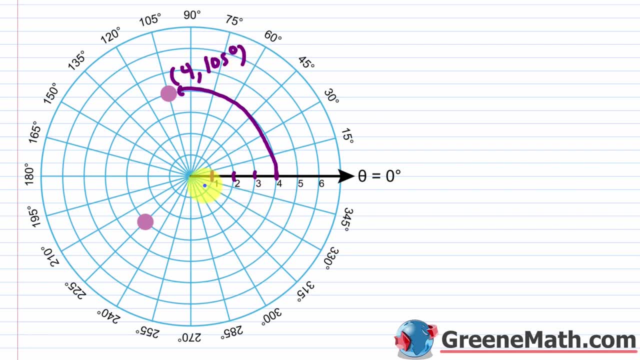 105 degrees. okay, Then for the other one we have the 3 comma: 225 degrees. So I'm going to step out and again I'm just going to swing around here to 225 degrees, And I know this is upside down. 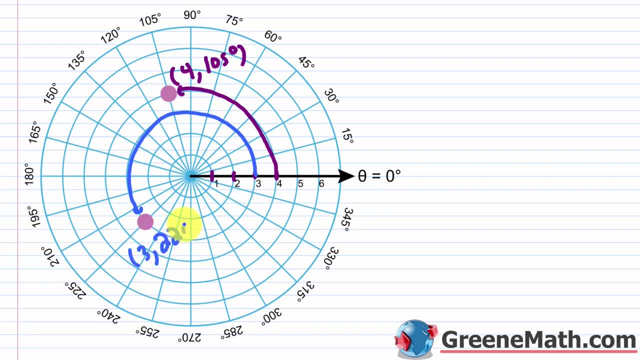 but you can still read it. So this is 3 comma, 225 degrees, like this. okay, So we've plotted those two guys. So now I want to think about: okay, if I had a little line segment that was drawn connecting those two points, I want the length of that line segment, which is the distance between 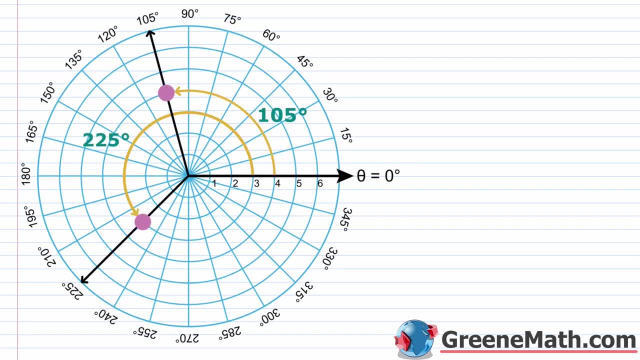 those two. okay, So the first thing we need is to figure out what is the angle between the two, okay? So, in other words, what is this angle right here? if I was to sketch this, what is that? Well, again, if you think about the whole, 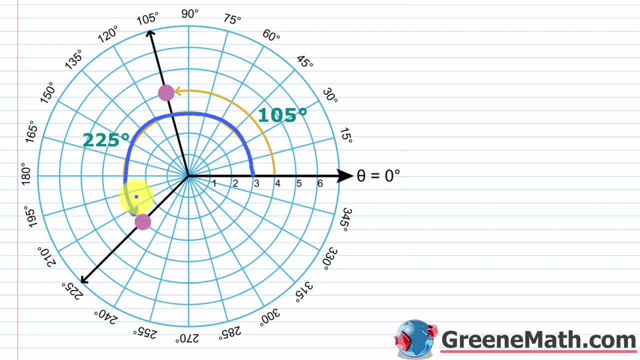 part here. let's say I start from here and I go all the way out here. that's a 225 degree angle. okay, But this angle here is only 105 degrees. okay, right there. So if I consider the fact that, 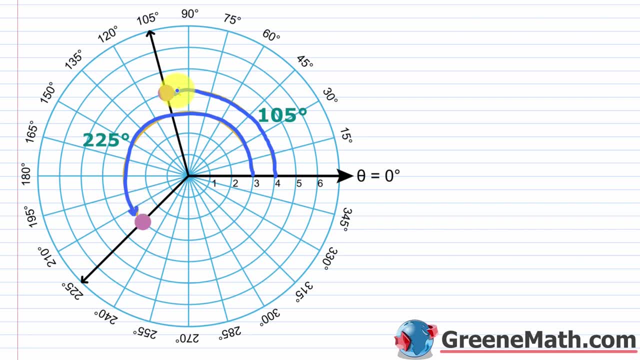 to go all the way around at 225 degrees. if I wanted to take this part out, okay, I would be excluding this from here, and I should probably do that in a different color. So if I took this part right here out, I would have the angle that I'm looking for. So if I took this part out, 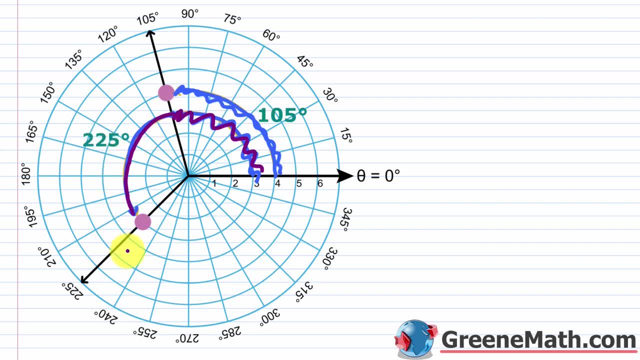 I would have the angle that I'm looking for, okay. So, basically, you're going to do this with subtraction. You can take the larger angle here, which is 225 degrees, and I could subtract away this smaller angle here, which is 105 degrees, okay, And this would give me 120 degrees. So 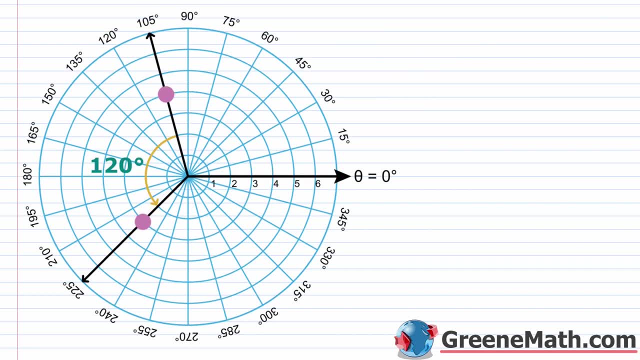 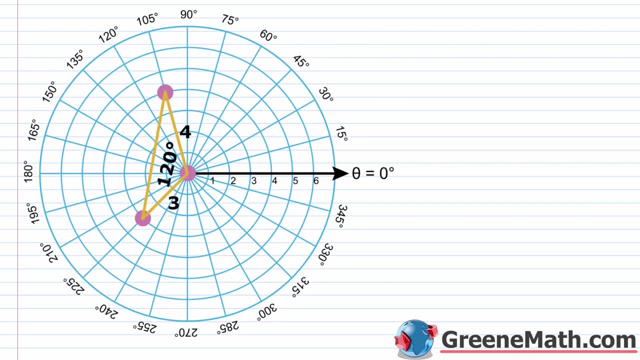 that's going to be my angle between these two guys. You can see, I've already made a little diagram for us with this. So again, this is just the angle between the two. okay, So we need this. Now we can set up a little triangle. once we know this, We already know that if we had 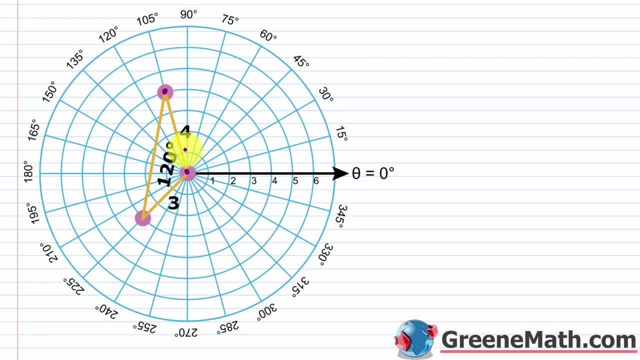 a little line segment, drawn from here to here, that the length of it would be four. right, Because this guy is lying on a circle with a radius of four. This guy right here is lying on a circle with a radius of three. okay, So this would be of length three. So we have a side of three. 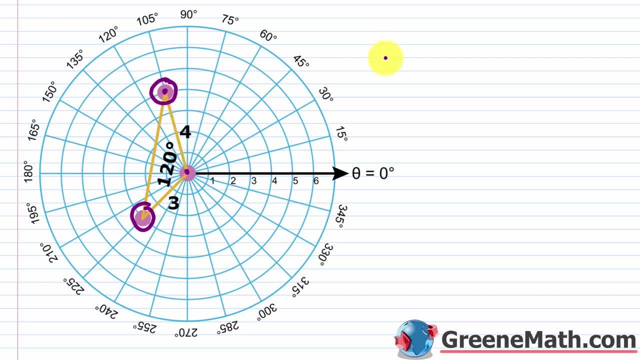 an angle of 120 degrees and a side of four. We have the side angle side, which allows us to use the law of cosines to find the missing sides. So let's just call this A Again. you can call it whatever you want. You can do A, B or C. I'm just going to call it lowercase a. 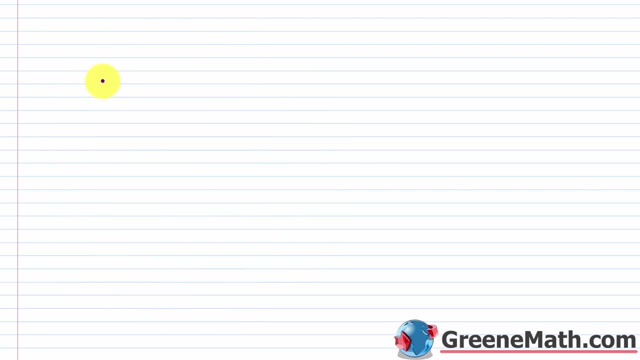 Okay. So let's come down here and let's remember that. let's say you were trying to find this lowercase a being squared, So side A, This is equal to remember. you're going to think about the B and the C that you know. So we're going to say: B squared plus C squared, then minus two times. 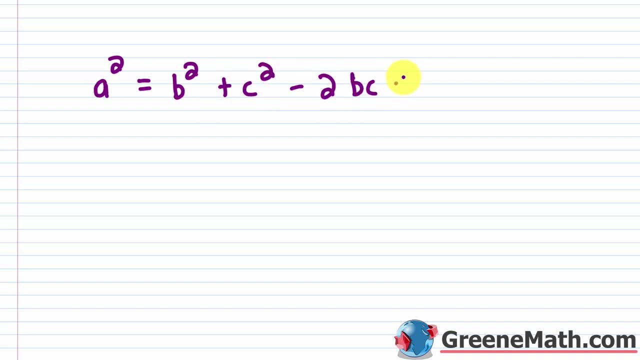 you're going to have the B times the C, okay, And then we're going to multiply this by the cosine, okay, of the angle you know. So it's always going to be opposite of this guy. So in this case, it's going to be the cosine of capital letter A, okay. In this case, it's going to be our 120. 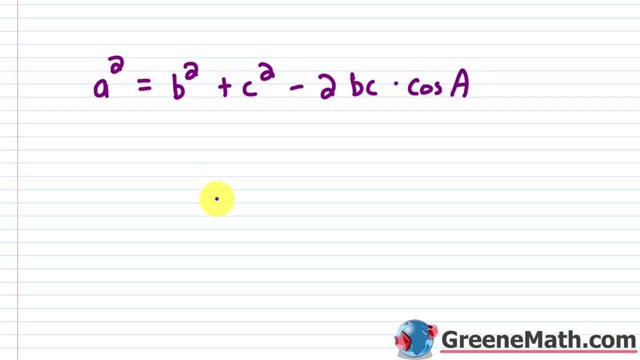 degrees. okay, So now all you have to do in this case is just plug in. I'm going to say that A squared- so A squared is equal to one of the sides- is going to be four, the other's three. It does not matter how you put it in there, and I'll show you that later on, But basically. 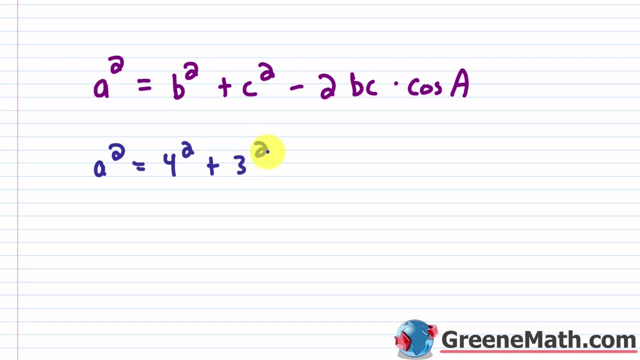 just go ahead and say: we have four squared plus three squared, okay, And I'll put minus. I'll go two times. I'll go ahead and say four and then times three and then times the cosine of 120 degrees, okay, So once you get it to this point, you're just simplifying, You can. 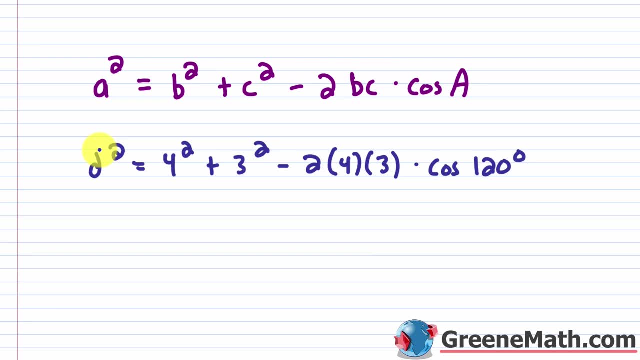 replace A with D, okay, Because you're trying to find the distance between the two. It doesn't matter, It's just a letter. So I'll say that, basically, my D squared is equal to four, squared is 16, then plus three, squared is nine. then minus, you're going to have two times four. 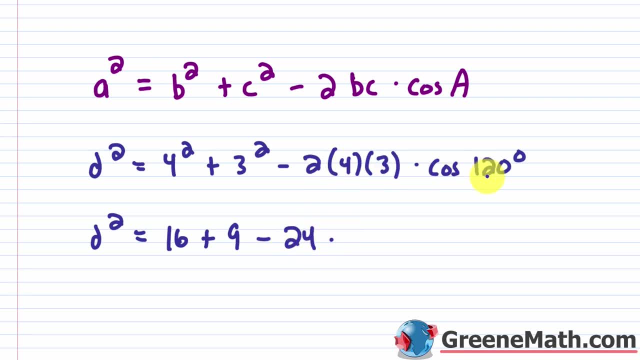 which is eight times three, which is 24, and then multiplied by the cosine of 120 degrees. Again, that's going to be in quadrant two. You have a 60 degree reference angle, So cosine of 60 degrees is a half. So cosine of 120 degrees would be negative one half, okay. So to simplify, 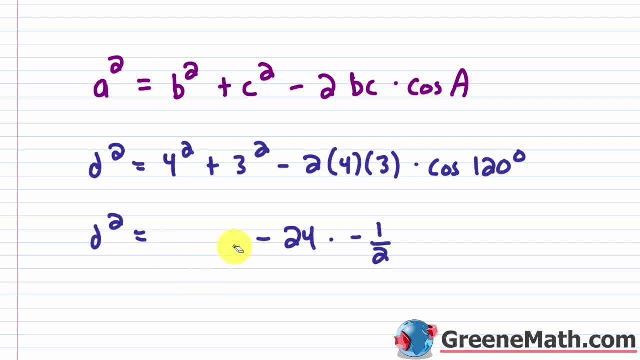 this: 16 plus nine is 25.. Let's just do it right here. We'll say: this is 25, and then this would cancel. with this, The negatives would also cancel. so this is going to be plus, And basically 24 divided by two is 12.. So I'll say this is 25 plus 12,. okay, Which is basically going to give. 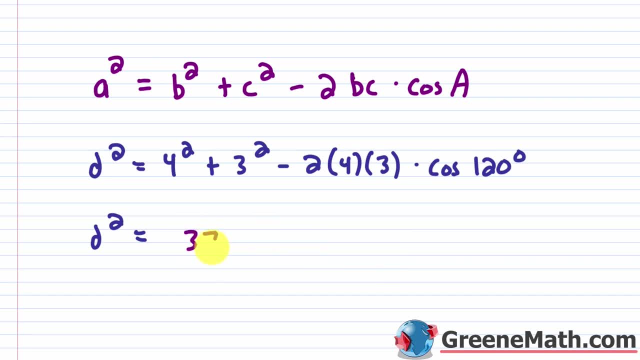 me 37.. So we have that the distance squared is 37, and if I want the distance, I'm just going to take the principal square root of each side and it'll be the square root of 37, okay, So basically, we've found that the distance squared is 37, and if I want the distance, I'm just going. 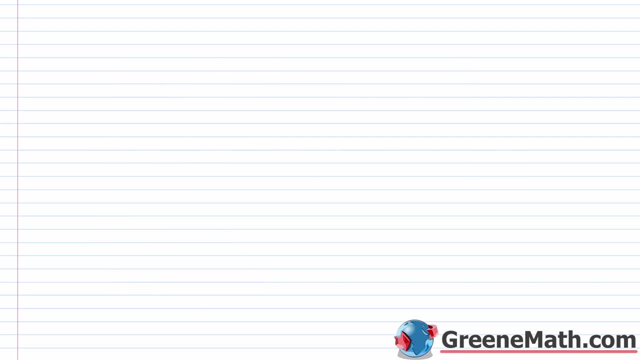 that the distance between those two points is the square root of 37.. Now how can we generalize what we just looked at? Let me write this again: We had a squared, but I'm going to call this d squared right. D, for distance, is equal to. we had basically our two sides that were known, So we 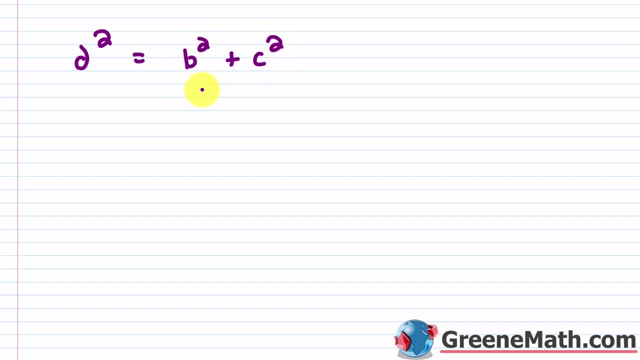 said b squared plus c squared. Let's go ahead and replace this, since when we have polar coordinates, we're going to have something like r sub one. let's say theta sub one, okay, And the r sub one is the length of a line, segment or a side of the triangle, And then we also have the r sub two. 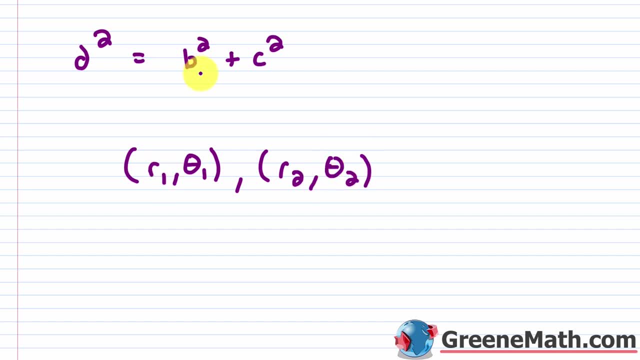 comma, theta, sub two. okay, So what we're going to do is we're going to plug in, instead of the b and the c, I'll go ahead and just say this is r, sub one. I'm going to put this in parentheses because 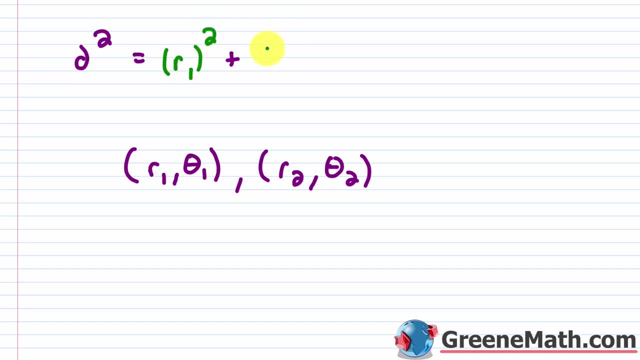 it gets kind of messy. So r sub one, that's being squared, And this one will be r sub two. this is being squared. It does not matter which point gets labeled as which, and I'll explain why that works out in a moment. okay, So then you're going to put the minus here. 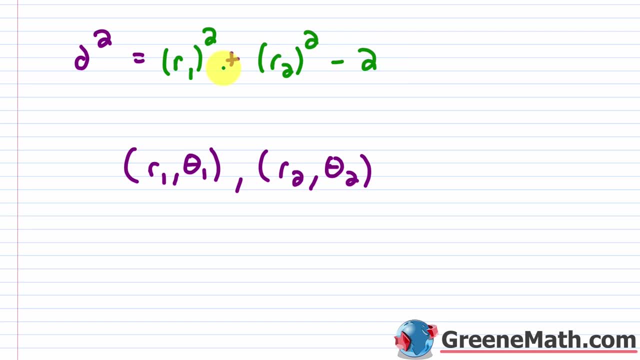 and then two times again. it's. these guys Remember with the formula it was two times. in this case it would be b times c. It's basically those two known sides. So I would say times r sub one, and then times r sub two, and then times cosine of the angle that you know. 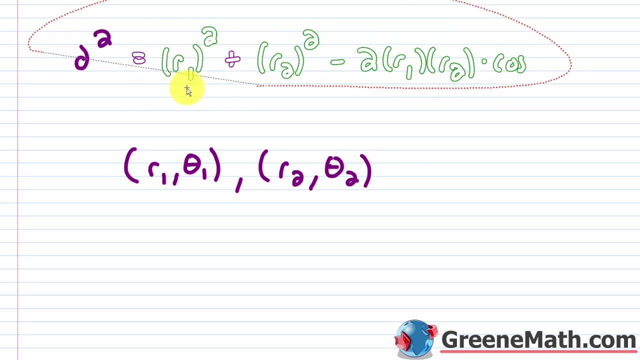 Now, in this particular case, remember how we found this. we subtracted okay. So I'm going to do is I'm going to say that I have theta sub two minus theta sub one. The reason it doesn't matter here is that, let's say, you end up with something that's negative. 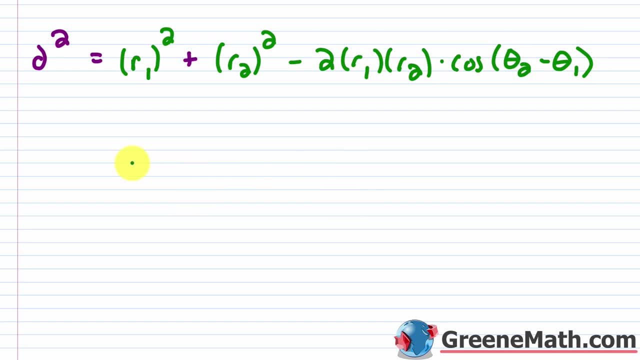 Remember, with cosine you have this negative angle, identity. So the cosine of negative theta- okay, if it ends up being negative- is the same as the cosine of theta, okay. So it doesn't matter if you produce a negative angle there, it's the same as if it would have been positive, okay, So 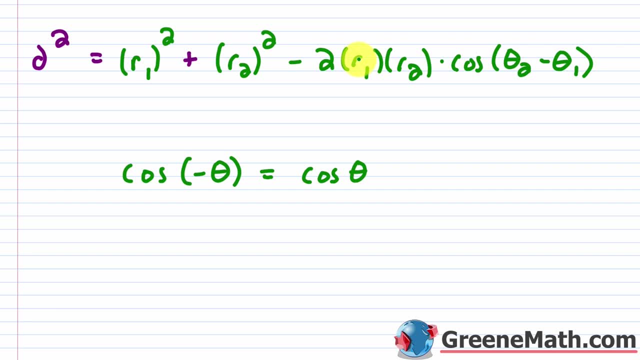 you will get the same result either way. None of this stuff matters in terms of the order, right? You're just doing some simple operations here, So the order that you choose the points does not matter. Very important, okay, So this would be our formula. Of course, you could take the square root. 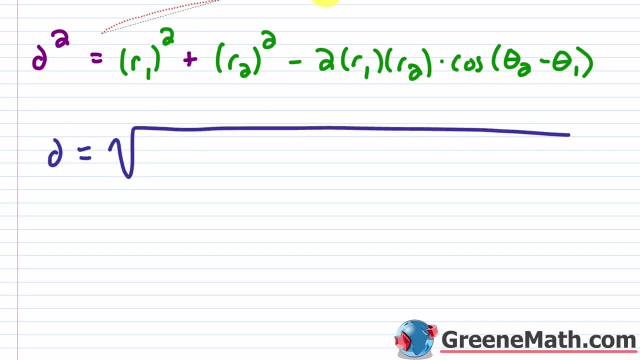 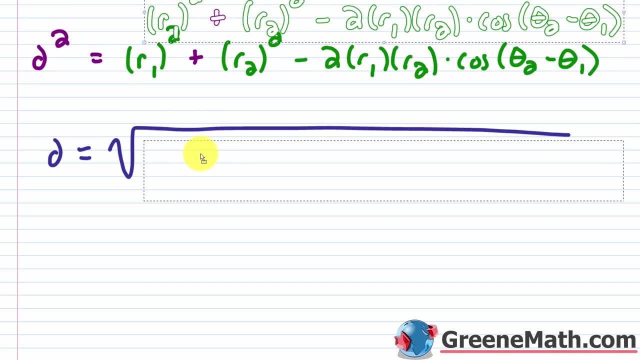 so you could say: D is equal to the square root of, and I could basically just copy all this. And let me go ahead and copy that real fast And let me paste this in And I'll just stick that underneath there So we don't have to write it. And let me just make that a little bit longer. 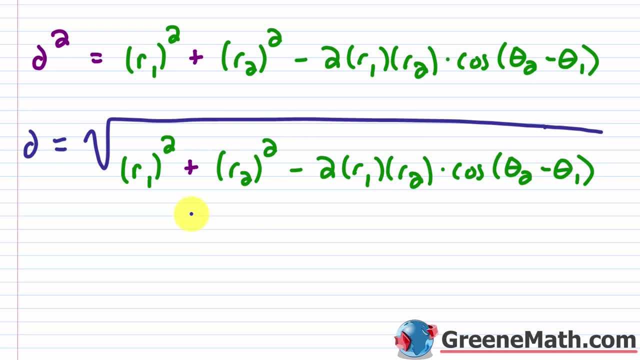 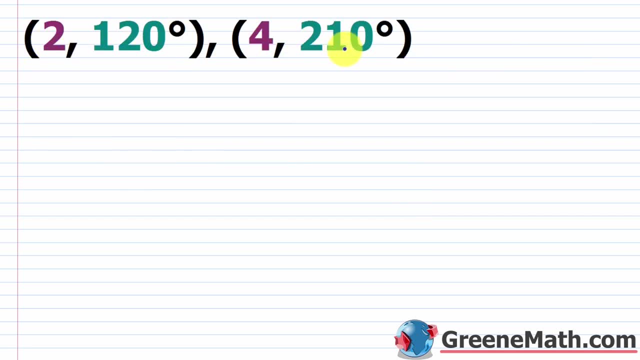 And I'll just slide this down a little bit so it fits on the screen, okay. So definitely something you want to copy down for your notes. And let's go ahead and just look at some examples. So we have 2,120 degrees and then 4,210 degrees. Again, you can label these however you want. 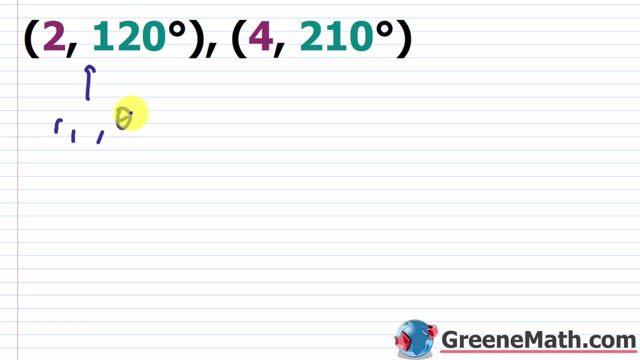 comes out the same way. So let's say this is R sub one and this is theta sub one. Let's say this is R sub two and this is theta sub two. So the distance between the two. let me go ahead and write it out a few times so you get. 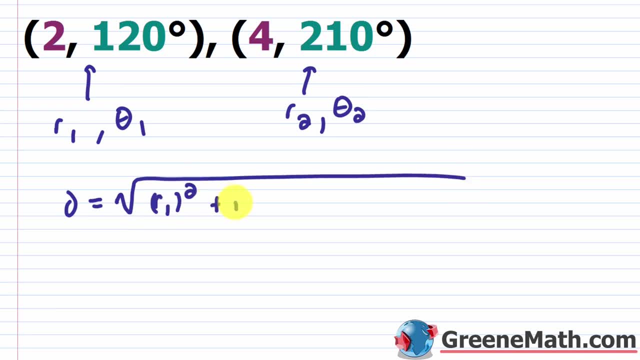 used to it. So R sub one being squared plus, you have your R sub two being squared, and then minus two times your R sub one, times your R sub two, and then multiplied by the cosine of the angle between them. So we're going to say theta sub two minus theta sub one. okay, So let's just go ahead. 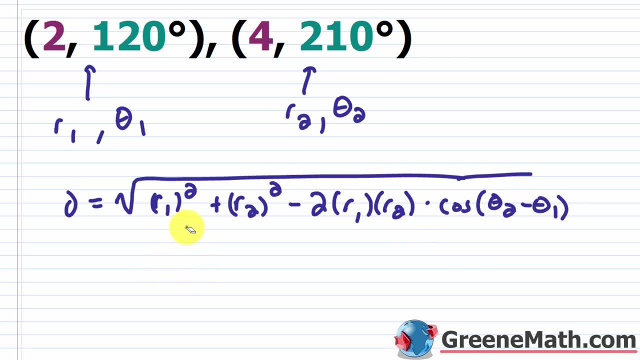 and plug in. We know that everywhere we see R sub one, we know that everywhere we see R sub two, we're going to plug in a two. So let's put two squared here and let's put two here, okay, And 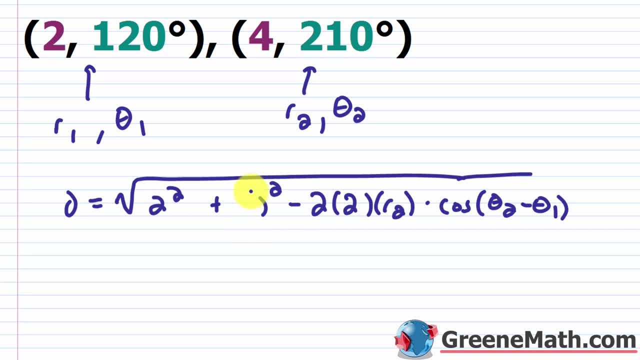 then everywhere we see R sub two, we're going to put four. So let's go ahead and put a four there- We don't really need parentheses there- And let's put a four there, And then, for theta sub two minus theta sub one, you're going to have 210 degrees minus 120 degrees, which would be 90 degrees. So 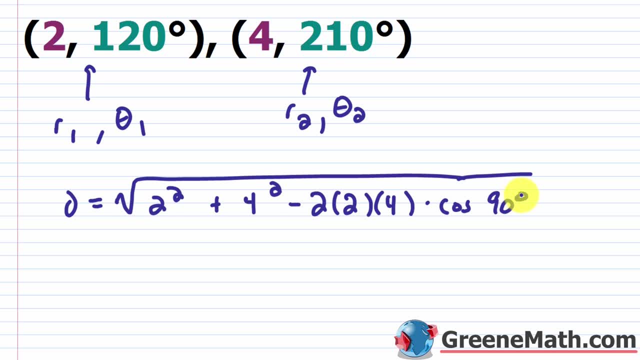 let's just go ahead and put cosine of 90 degrees. Now, most of you know that cosine of 90 degrees is zero, So you could basically get rid of that. So let's go ahead and put cosine of 90 degrees, So you can just erase this. You don't even need it because you'd be subtracting away zero. 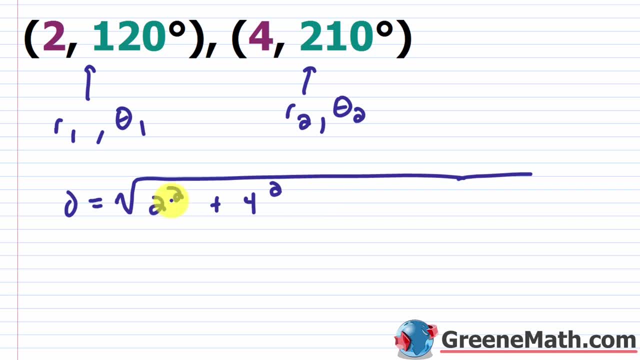 which doesn't change anything. So here we're just going to have the square root of two squared plus four squared. So two squared is obviously four and four squared is obviously 16, okay. And then if we add those together we would get 20, okay. So the square root of 20, remember, you can. 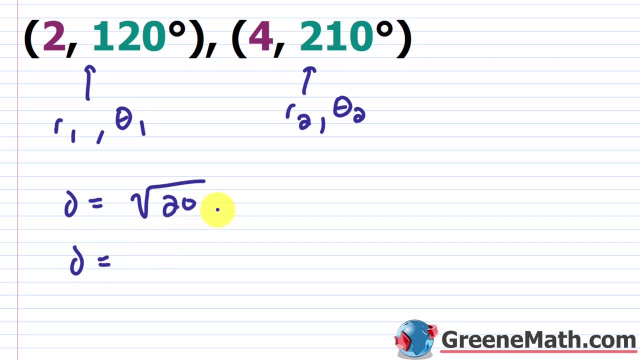 simplify this. We could say: d is equal to. this would factor into four times five and four is a perfect square, right? So basically, I can say: this is two times four and four is a perfect square. okay, So that's going to be my answer for the distance between these two points. Again, if you, 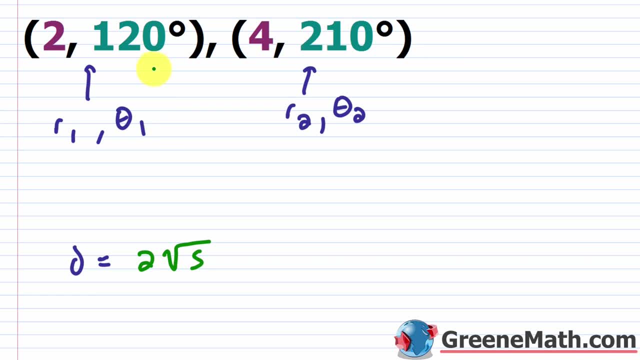 change up the ordering. pause the video. you can see this on your own. The only difference is you're going to end up with the cosine of negative 90 degrees, And you could say that the cosine of negative 90 degrees is equal to the cosine of 90 degrees In each case. let me put my degree symbol. 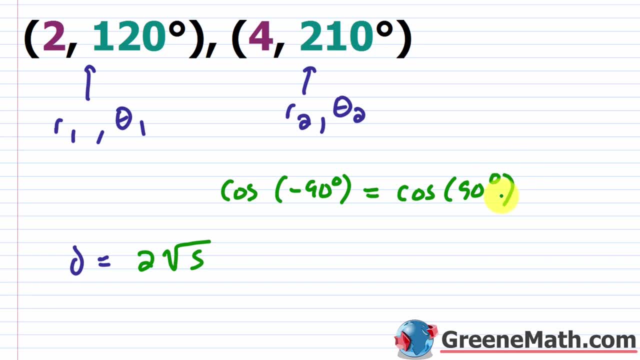 in there, so that's better. In each case, you're going to get zero, okay, So remember this identity here. Let's take a look at another example. Here we'll work with some radians, So let's just go ahead and label this as r sub one, comma theta sub one. Let's label this as r sub two. 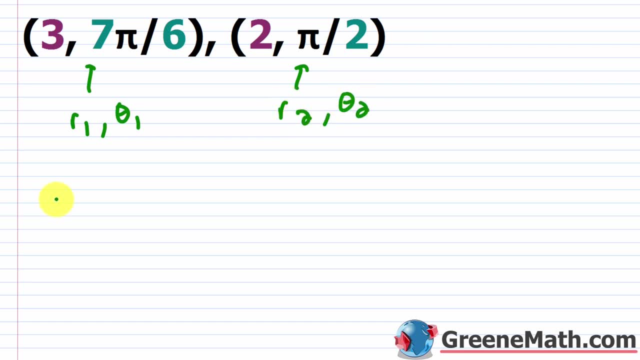 comma, theta sub two. And again I'm just going to plug into the formula. So the distance is equal to the square root of. let's just go ahead and say r sub one is three. So we'll say three squared plus r sub two is two. So two squared, then minus two times, you're going to have r sub one. 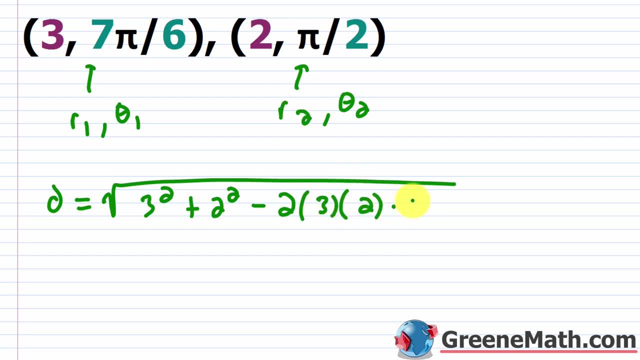 which is three times r, sub two, which is two, and then times. the cosine of this was a little bit tricky, because you do have to work with fractions here, So let's just go ahead and do this. off to the side, I'm going to have pi over two and I'm subtracting away seven pi over. 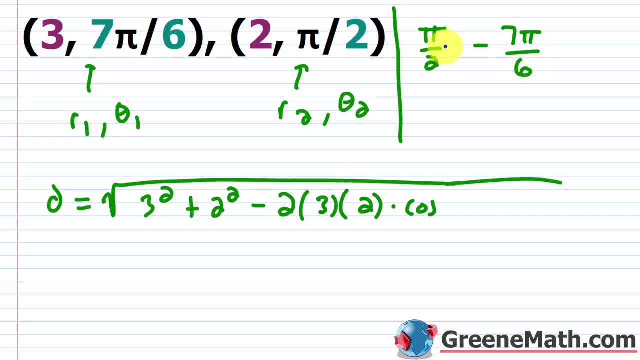 six. okay, I need a common denominator, so I'm going to multiply this by three over three, So this would be three pi over six. Three pi minus seven pi is negative four pi, So this would be negative four pi. and then over that common denominator of six, And of course you can. 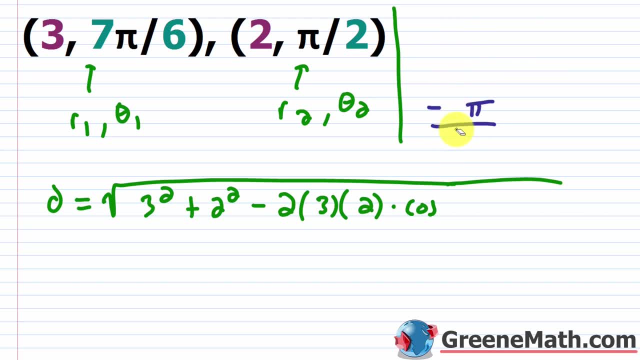 reduce this fraction, This would end up being negative two pi over three. okay, So negative two pi over three. let's write that in here: negative two pi over three. So this would be negative two pi over three. okay, Now, if you want to remember, because of the negative angle. 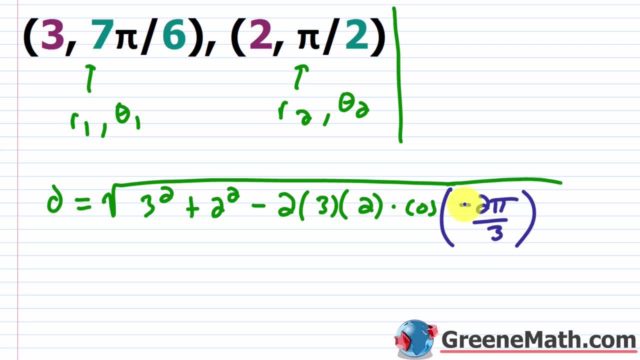 identity for cosine. this is the same as if I had cosine of two pi over three. So you can just get rid of the negative there. That way it makes it a little bit easier if you're working off the unit circle And from here I can just go through and evaluate things. Three squared is going to be nine. 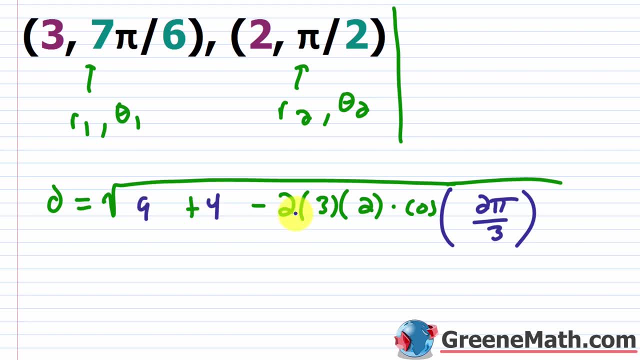 and two squared is going to be four And basically you have two times three, which is six times two, which is 12.. So this is a 12 here. Nine plus four is 13,. let's just go ahead and do that real quick, And essentially the cosine of two pi over three. 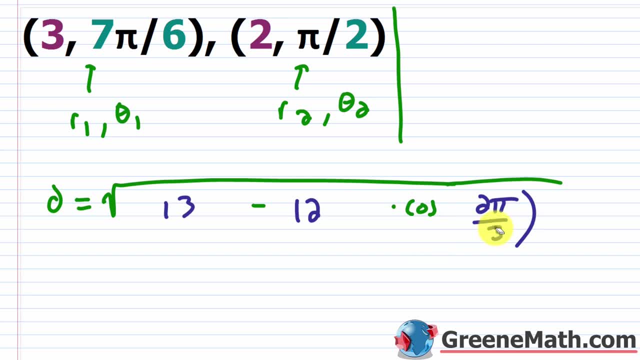 remember, two pi over three is 120 degrees And we already know the cosine of 120 degrees is negative a half. So this is times negative one half. I like to wrap this in parentheses because basically you want to do this operation first. I know that's pretty obvious for most people, but I don't want. 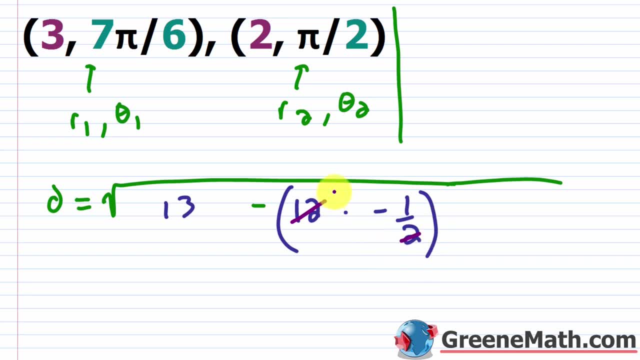 you to get confused as to what's going on. So this is going to cancel with this and give me a six here. So basically you would have a negative six, right? So what you end up with here is minus a negative six, which is like adding six. So 13 plus six would be 19.. So basically here. 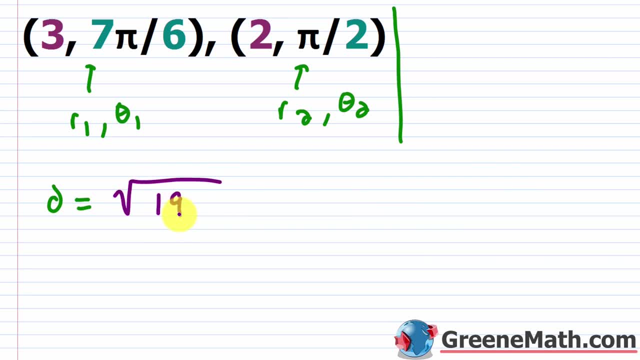 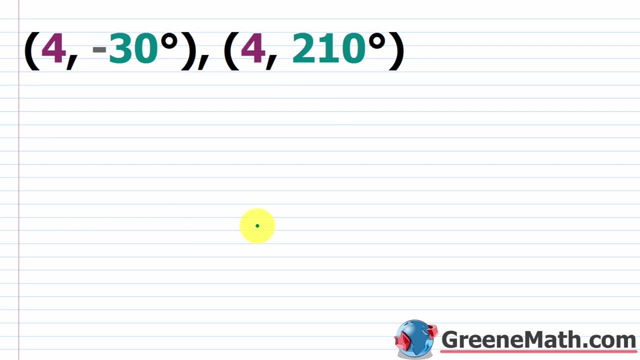 the distance between these two points would be the square root of 19.. All right, what I want to do now is look at two different examples where you have these negative angles and also the negative r values. This is a bit tricky for students to understand. you can basically just take what 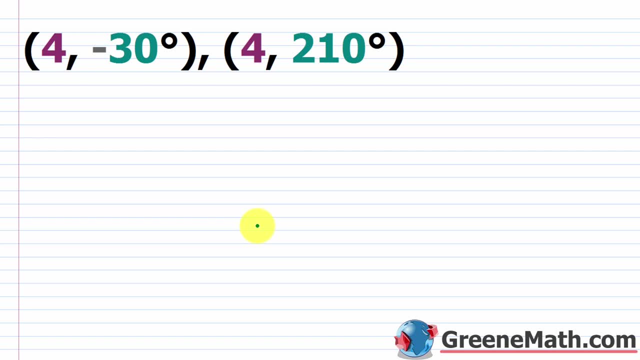 you have okay as it's given and plug it into the formula and it's still going to work, Okay, So I'm going to use this directly as it's given, then I'm going to use it as a negative, And then 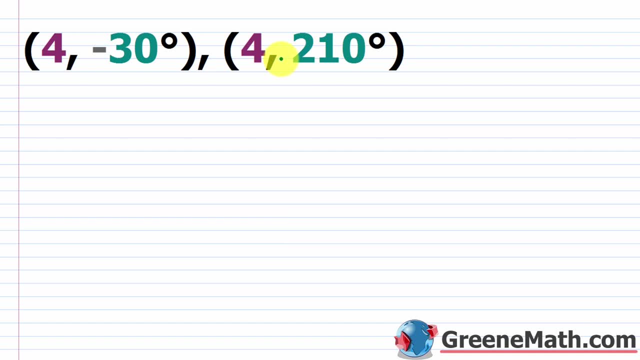 I'm going to change it over and I'll show you why it doesn't make a difference. So, first and foremost, we have four comma negative 30 degrees. Let's say this is our first point. Again, it doesn't matter how you label this, I'll go ahead and say this is r sub one comma, theta sub one. 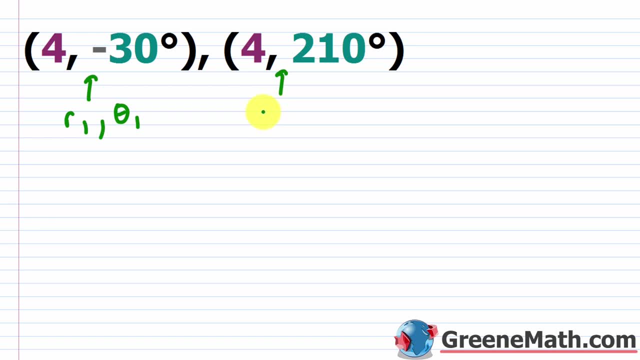 And then let's say this: four comma, 210 degrees. Let's say that's the second point, So r sub two comma, theta sub two. Okay, So from here we just plug into the distance formula. So d, the distance between the two points is the square root of you're going to take this guy and square it. 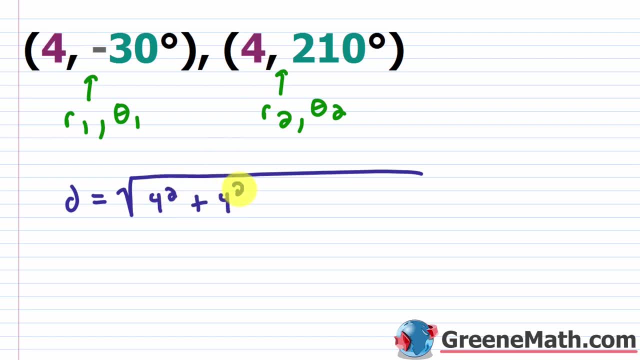 so four squared, Plus, you're going to take this guy and square it. so four squared, And then minus, you have your two times this guy times this guy. So four times four, Okay. And then times the cosine of the angle between them, Okay. So what? I'm going to go ahead. 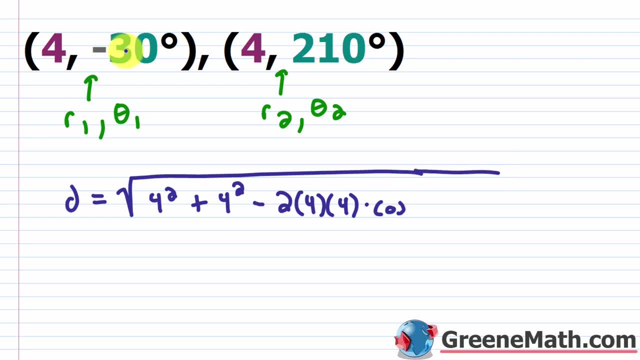 and do is just say it's 210 degrees minus a negative 30 degrees. Okay, Remember, minus a negative is plus a positive. So 210 degrees minus a negative 30 degrees, Okay, And let me go ahead and close that down And from here we're just going to simplify, Okay. So I'm going to say 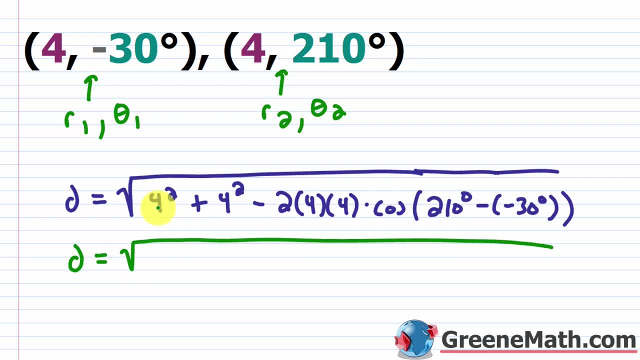 the distance between the two is equal to the square root of this would be 16.. And this would be 16.. 16 plus 16 is 32.. So let's write that, And then, minus, you have two times four, which is: 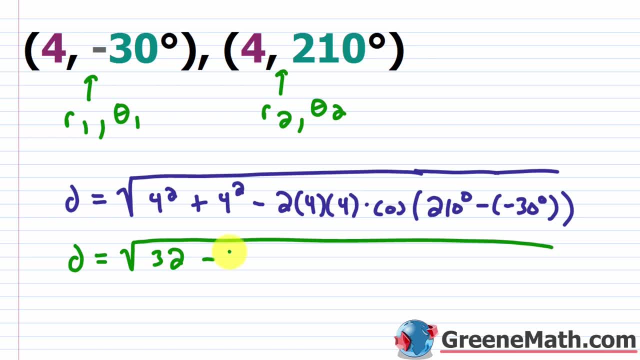 going to be eight, And then times four again, which is going to be 32.. Okay, So you have 32 there, And then times, you're going to have the cosine of 210 degrees minus a negative 30 degrees is 240. 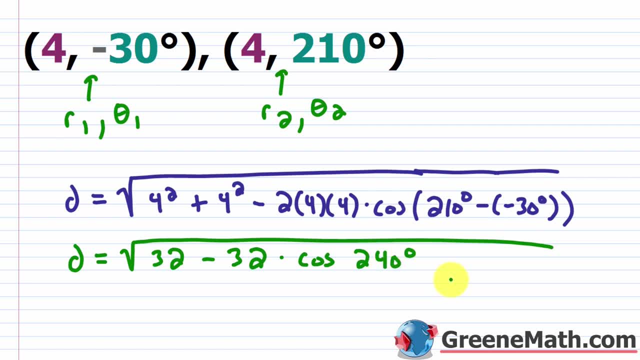 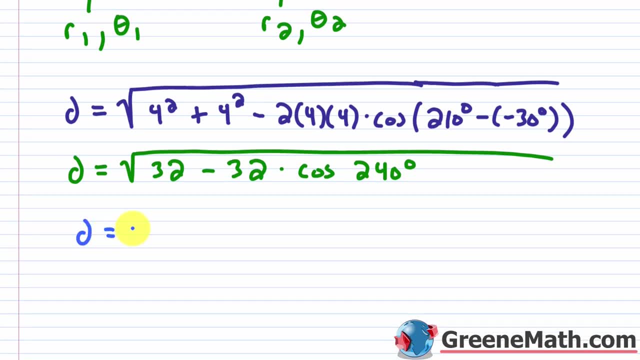 degrees. So let me put 240 degrees there, Okay. So let me just scroll down and get a little bit so we can fit everything on the screen. So I'll say: the distance is equal to the square root of the cosine of 240 degrees. Again, this is going to be in quadrant three now And you're going to 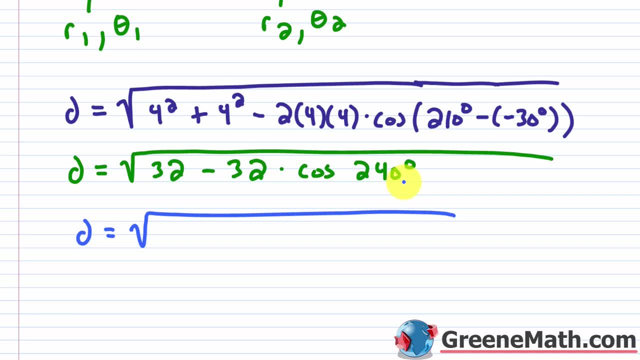 have a 60 degree reference angle. So this is going to be negative one half. Okay, So you would have 32 minus you'll have 32 times negative one half Again. if you want to make this clear, it's not necessary. You can wrap this in parentheses. It's kind of up to you. So I'm 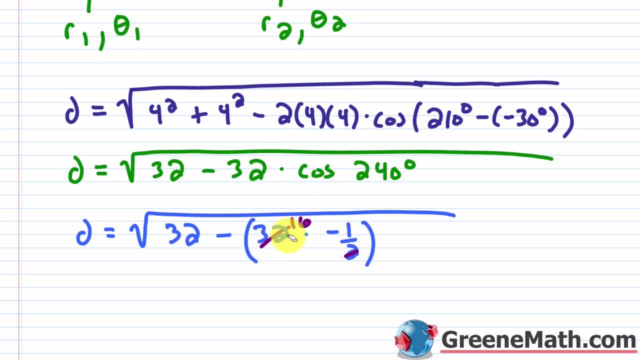 going to cancel this with this and put a 16 here. So basically, you would have 32, minus a negative 16.. That's why I like the parentheses there, So it makes that clear. So, basically, 32 minus a negative 16 is 32 plus 16, which is 48.. Okay, So this is the square root. 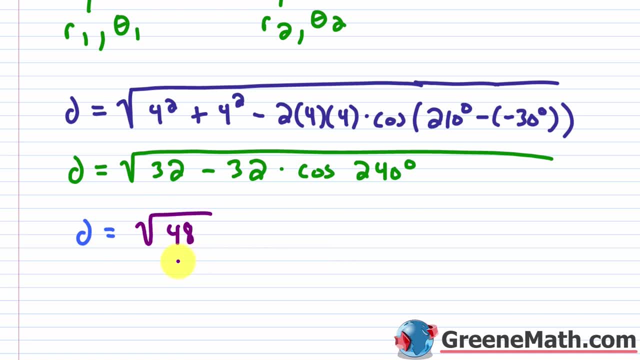 And let me make this a little bit smaller- This is the square root of 48.. Of course, 48 is going to be 16 times three, and 16 is a perfect square, right, It's four times four, So you can go ahead. 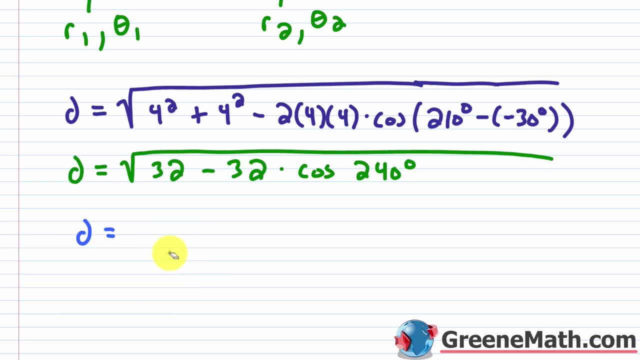 and write this as four times the square root of three. Okay, So I'm going to say the distance is four times the square root of three. Now I want you to pause for a minute because some of you who try to plot this, if you go back up and you think about these points here, 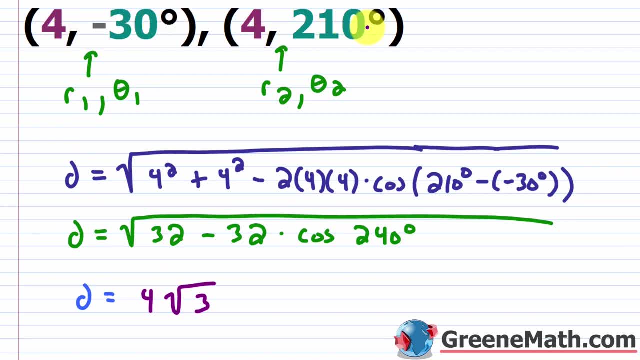 four comma negative 30 degrees and four comma 210 degrees. If you think about the angle between them, it's not 240 degrees, It's going to be 120 degrees. So why in the world did we get the right answer? And I'll show you in a moment that if you do it the other way, you'll still get the same. 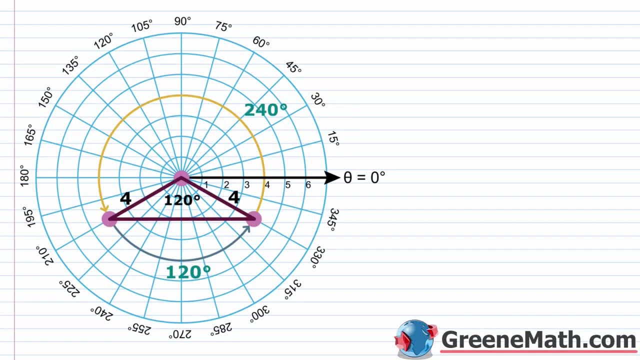 thing. If we go to a little diagram here, you'll see that I've kind of drawn everything out. If you start at this point here, let me label this, So everything's crystal clear Right here- could be thought of as either four comma 330 degrees or, if you're rotating this way, 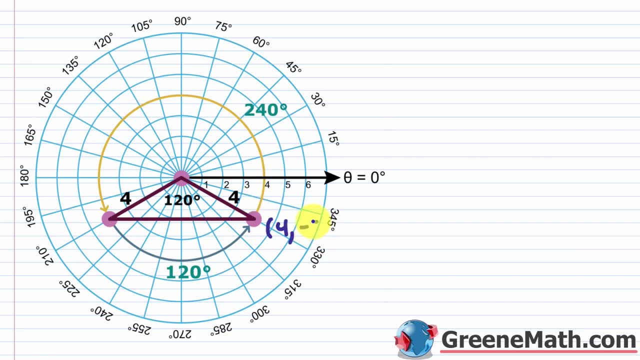 clockwise, you could say that it's four comma negative 30 degrees, Okay. And then this point over here, you could think about it again as four comma 210 degrees, Okay. Four comma 210 degrees like this, Okay. So if we think about the angle between these, you can just look here. I've already 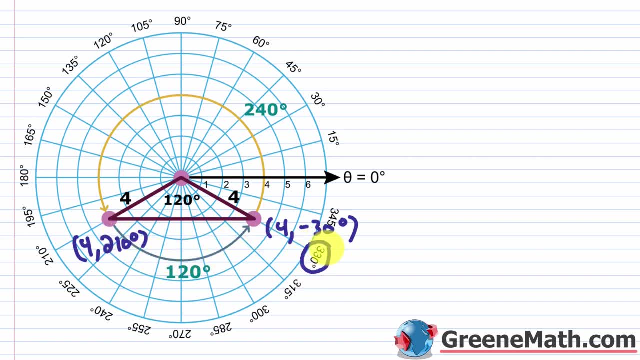 kind of done this for you. I've already done this for you. I've already done this for you, I've already done this for you. But essentially, if you start at this 330 degrees and you subtract away the 210 degrees, you can see this angle between them would be 120 degrees. Okay, The angle on the outside. 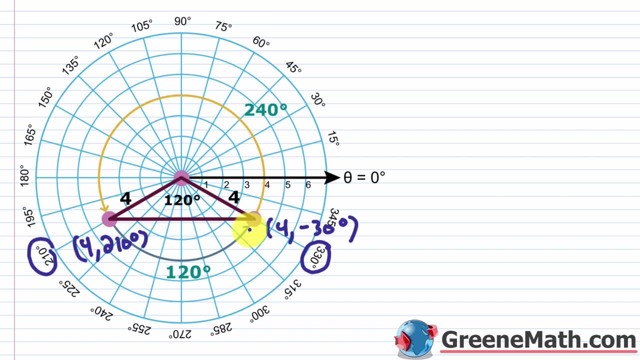 is going to be 360 degrees, one full rotation minus this 120 degrees, which is 240 degrees. Okay, So that's, if I started here and I rotate along the outside there, Okay, So that's 240 degrees. Okay, So we see that the angle should have been 120 degrees. So what in the world? 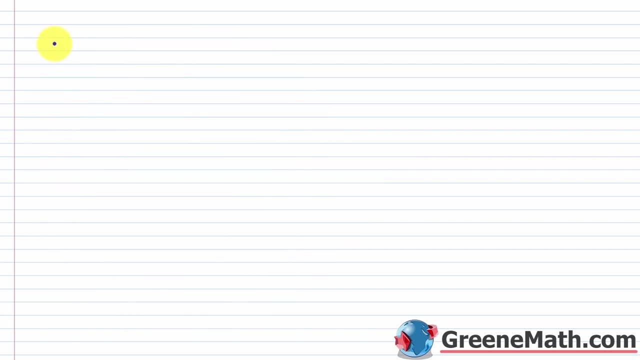 is going on. Well, it turns out that we have a little identity And it states that the cosine of, let's say, 360 degrees minus some angle theta- okay, whatever it is- is going to be equal to the cosine of that angle theta. So this is exactly what we just came across. We see that the cosine 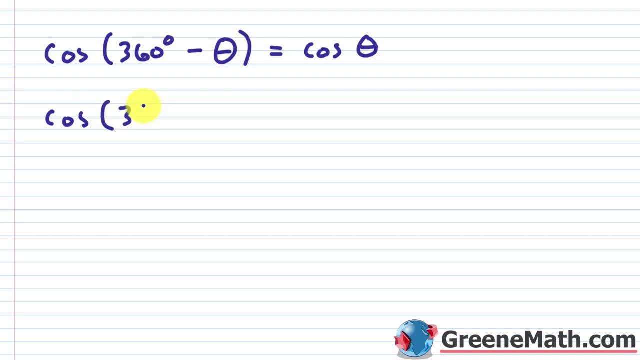 of. let's say theta is 120 degrees. So 360 degrees minus 120 degrees- okay, would be equal to the cosine of 120 degrees. This, right here, would end up being 240 degrees. So the cosine of 240 degrees is equal to the cosine of 120 degrees. 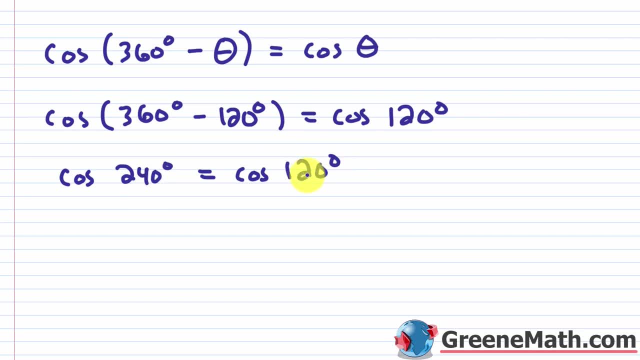 Okay. So it does not matter if I punch this in as 120 degrees for the cosine or 240 degrees. that value is the same, Okay. So when you go through and do your calculation, you're going to get the same answer, whether you work with it as is or you do a little conversion. Okay, 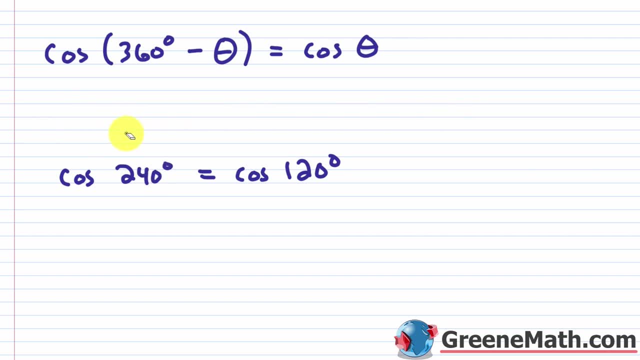 Now, this little identity here can be quickly proven using the difference identity for cosine. Okay, So if you want to go through that, you could basically say that this guy right here- let me erase this real quick- And we'll go ahead and say that this is what this is going to be- the cosine of the first guy. 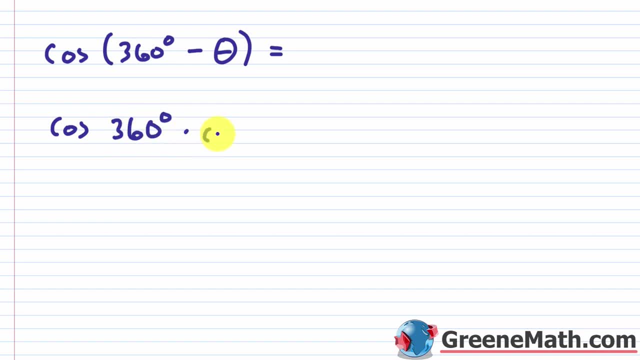 So 360 degrees, okay Times. the cosine of the second guy, So that's theta. Then remember, with the cosine difference identity, the sine is going to be opposite, right? So I'm going to make this a plus And then I'm going to go ahead and say, now that I have the sine of this first guy, 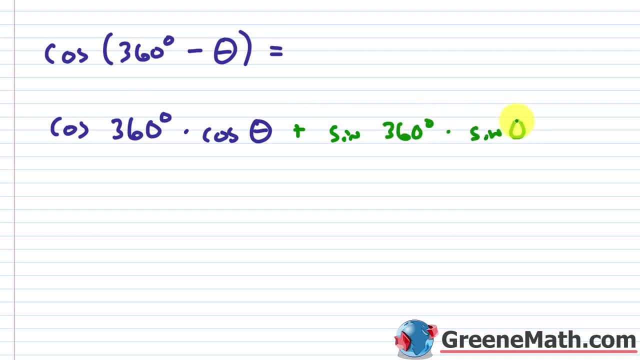 the 360 degrees and then times the sine of theta. Now I know the sine of 360 degrees is the same as the sine of zero degrees And the sine of zero degrees is going to be zero, right, So you can basically get rid of this. This is going to be. 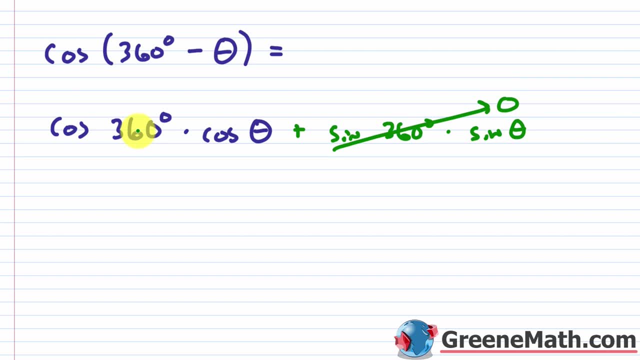 zero, And the cosine of 360 degrees is the same thing as the cosine of zero degrees, And that's going to be one, So you can get rid of this. This is a one. So basically, what you're left with here is one times the cosine of theta, which is just the cosine of theta. Okay, So that proves that. 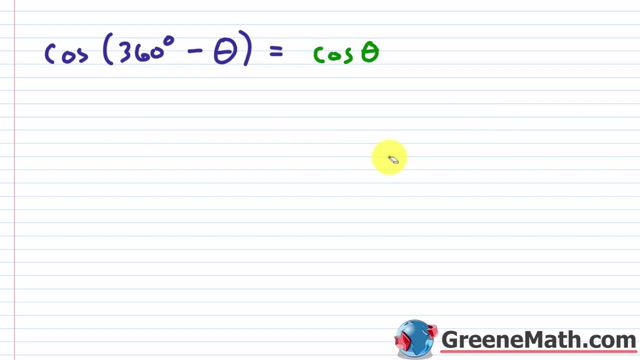 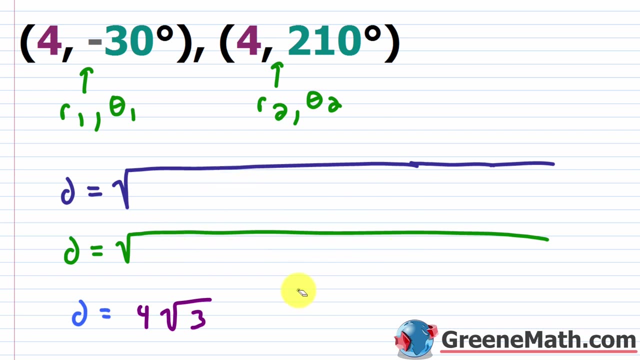 little identity there. We can get rid of this and go back to this form. And let's go back now And let's see what would happen. Let me go ahead and erase this. We'll keep this kind of here for now. Let's see what would happen if we converted this over Instead of having four comma negative. 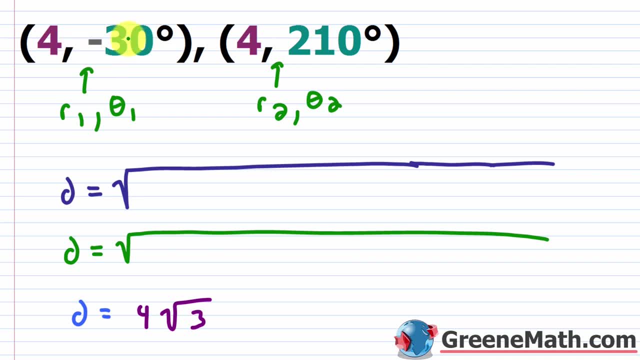 30 degrees. let's add 360 degrees and say that our other point is now going to be- and I'll just write this over here- We'll say it's four comma 330 degrees. Okay, So I'm just going to put this. 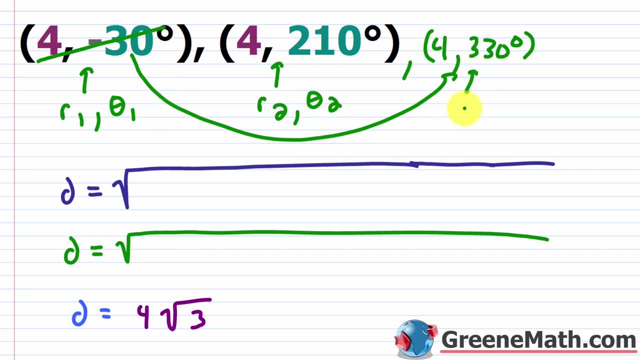 over here and just line this out for a moment And I'll say: this is my R sub one comma, theta sub one, And maybe we can just erase this. And then I'll say: this is my R sub one comma, theta sub one. 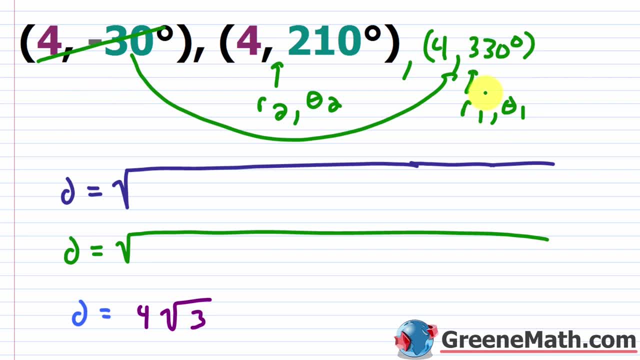 Just so it's clear what we're doing. And so, in this particular case, what would we do now? Well, we're going to say that we still have the same four squared, plus four squared, and then, minus two times, you have your four times four. Okay, So that part's all the same. 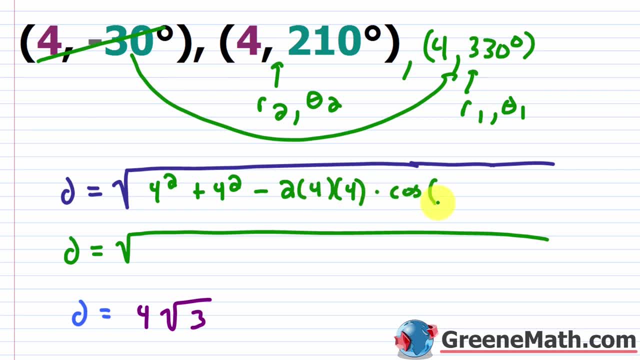 And then times the cosine of this part would be different. So basically you have your 210 degrees minus your 330 degrees, which is negative 120 degrees. Again, remember, because of your negative angle identity with cosine, You could just make this positive 120 degrees. Okay, It's going to be the same thing. 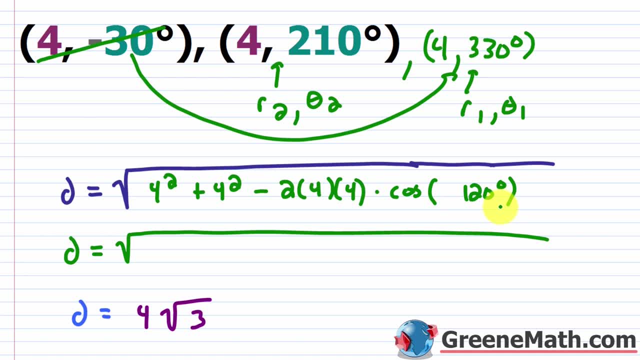 And essentially we already know that the cosine of 120 degrees and the cosine of 240 degrees will be the same right, We just saw that identity, So we know we would get the same answer. So we can go through here and just say, okay, well, this would be 16 plus 16.. Again, that's 32.. And then 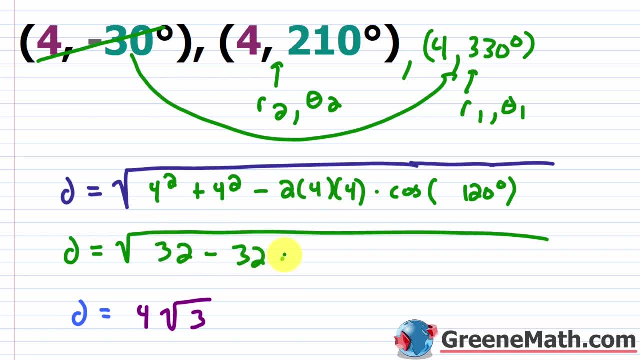 minus, you'd have two times, basically 16, which is 32.. And then times the cosine of 120 degrees, we know, is again negative one half. Okay, So you can wrap this in parentheses, same thing we did before. This would cancel with this and give me 16.. So this is negative 16.. Again, you get 32 minus a. 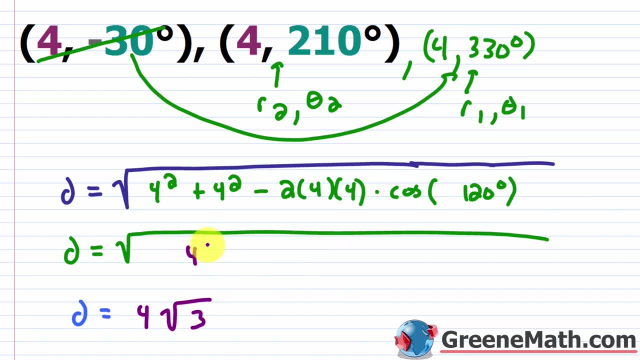 negative 16,, which is going to be 48.. Okay, So we end up simplifying this. We get: the distance between the two points is four times the square root of three. Okay, So it doesn't matter if you end up with a negative angle. you can work with your formula either way. Okay, Let's look at an example. 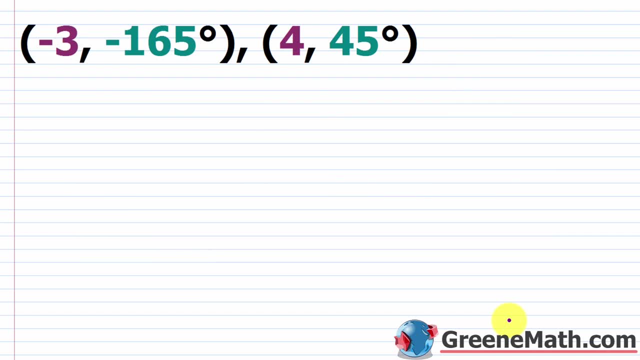 with a negative R value. So again, you have the choice of working with it, as is. Some people tell you to convert it. If you plug it into the formula, you will get the right answer. Okay, So if you have negative, three comma negative, 165 degrees, and then four comma 45 degrees, if you wanted to, 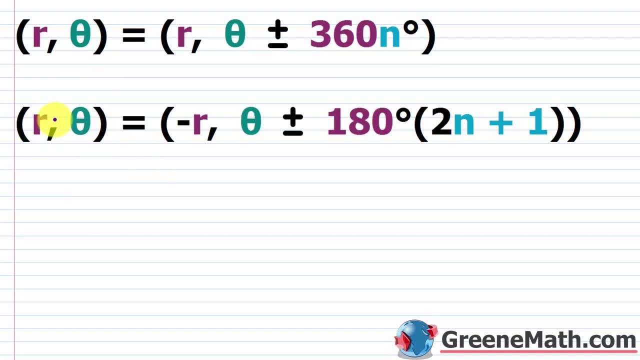 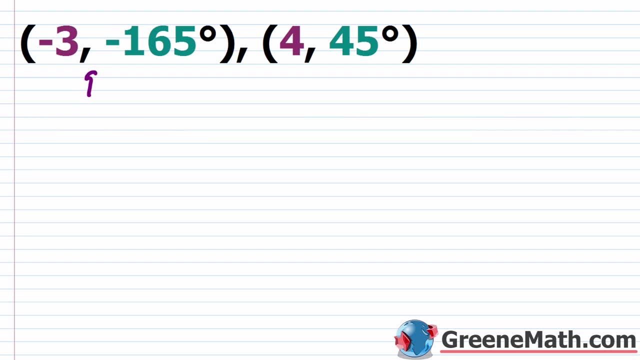 remember the little formula: if you have R and negative R, what you have to do is add 180 degrees to that. Okay, So that's how I could change this over. I could say that this same point could be located by saying: I have three comma at 180 degrees to this. this would be 15 degrees, Okay. 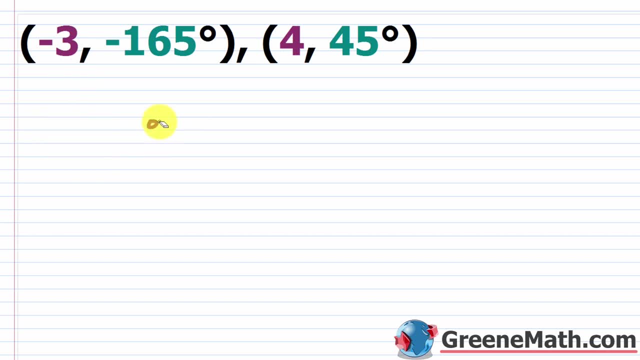 So you can use either one. Let's go ahead and use the first one And I'll show you it works the same either way. So the distance is equal to the square root of. let's call this point one, So R sub one, comma, theta sub one. let's call this point two, So R sub two, comma, theta sub two, And again, all I'm 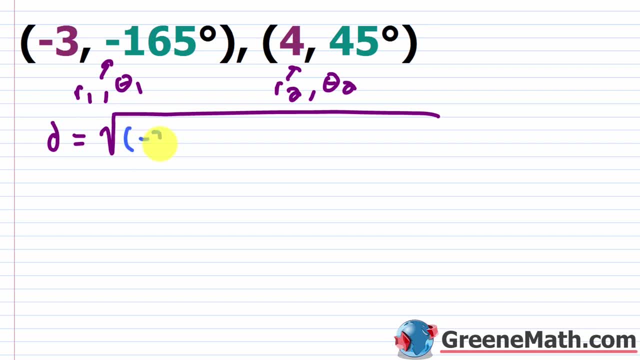 going to do is just plug in. So I'd have negative three, So negative three- be careful there- being squared, Plus you'd have four being squared, and then minus two, times negative three, Okay, Times four, and then times the cosine of if you subtract 45 minus a negative 165, that's like 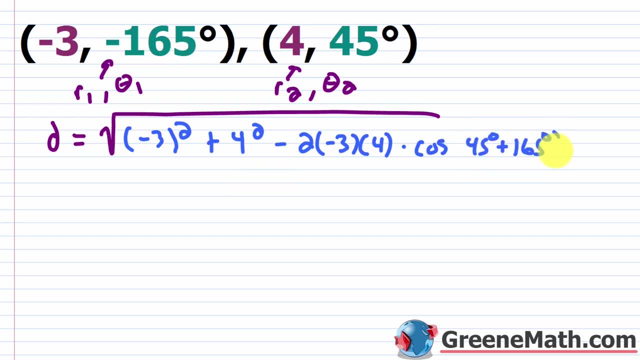 45 plus 165.. Okay, We put my degree symbols in there. So that's going to give me 210 degrees. Okay, So this is 210 degrees. Let me extend this a little bit over, All right, So let me put here. 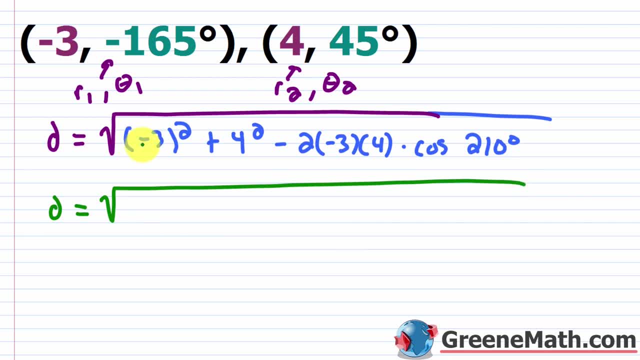 that the distance is equal to the square root of. if I square negative three, I get nine. If I square four, I get 16.. If I add nine and 16 together, I'm going to get 25.. Okay, So that's pretty simple. 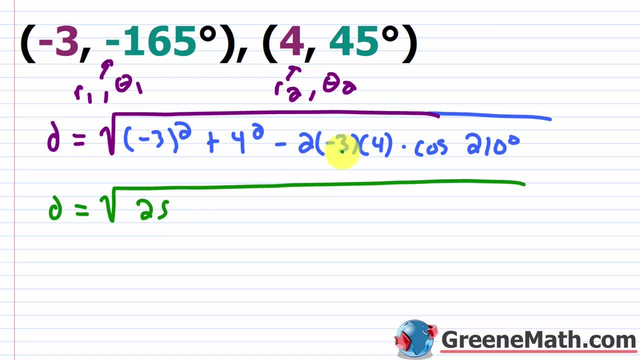 here. What I'm going to do is I'm going to say negative two times negative. three is positive six, and then positive six times four would be positive 24.. So let me put plus 24 times the cosine of 210 degrees, Now 210 degrees. 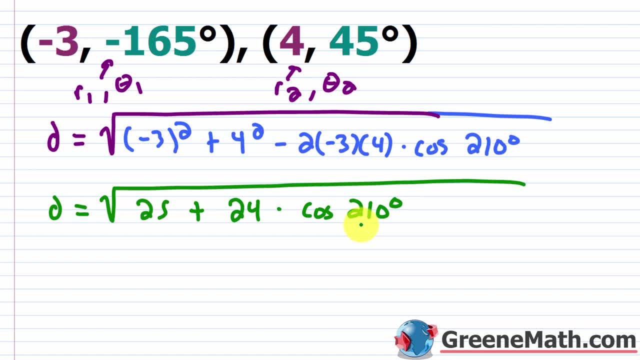 that's going to be in quadrant three. Okay, So cosine is negative and it's based on a 30 degree reference angle. Okay, So the cosine of 30 degrees is square root of three over two And because we're in quadrant three, this would be negative. So I'm going to say this is the negative of the. 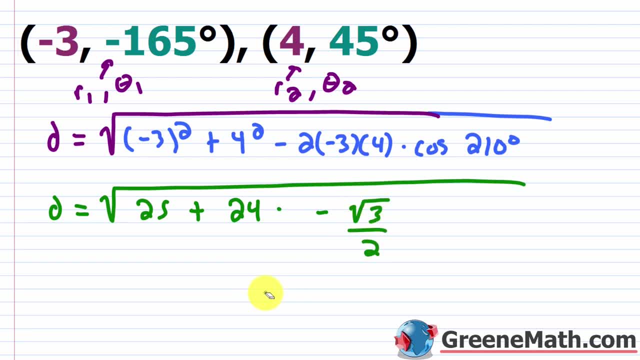 square root of three over two. Okay. So if you multiply these together, what's going to happen is this: would cancel with this and give me a 12.. Okay, And it's going to be negative. So I might as well just write minus and I'll say 12. 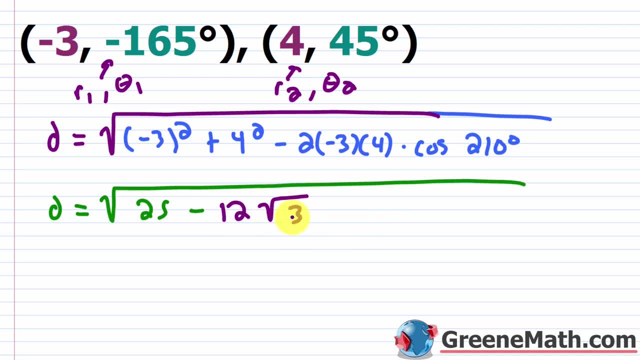 times the square root of three. Okay, Times the square root of three. Now you can approximate this if you want. If you want an exact answer, this is going to be it All right. So let's work with this point. I'll show you it still works. So we'll go ahead and say: change that R value. 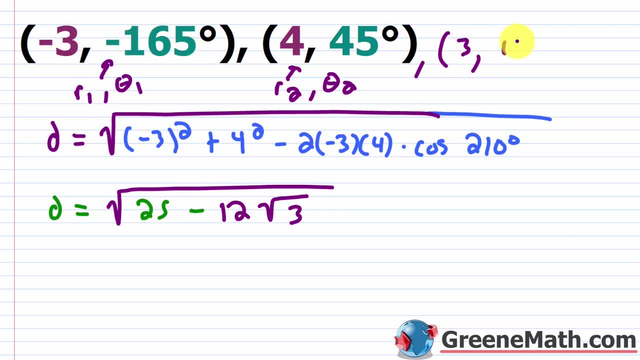 to positive at 180 degrees. to negative 165 degrees, That's 15 degrees. Let's line this all out. Let's get rid of that And I'll label this as R, sub one comma, theta. Okay, So if you plug in here, the sign's going to change, and here the sign's going to change. 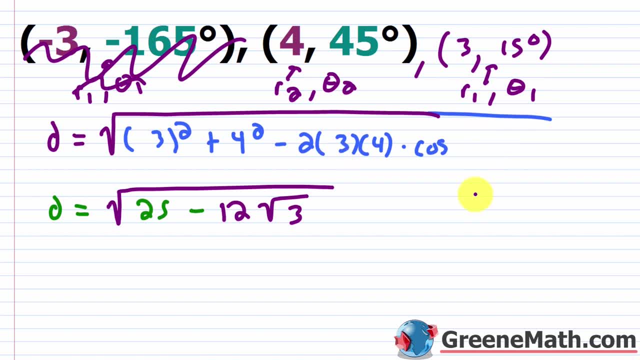 Okay, And this is going to change. Everything else would be the same, right? So basically, what you'd have here is inside. Now you do 45 degrees minus 15 degrees, Okay, And that's going to give me 30 degrees. So I want you to notice that a moment ago, we had the cosine of 210 degrees. 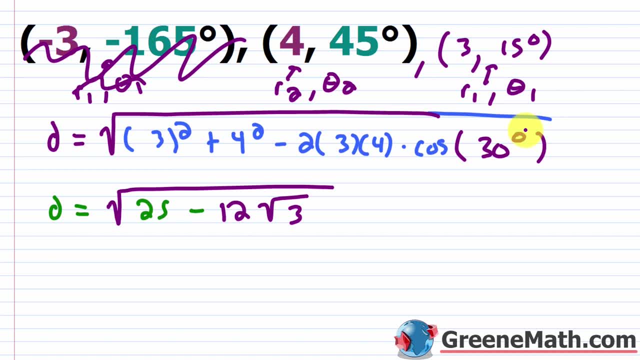 Okay, And essentially this had a 30 degree reference angle, but this guy is positive and the other guy's negative. But notice that you have a sign change here. Okay, Before you had negative two times negative three. Now it's negative two times positive three. Okay, So I'm going to show you a little. 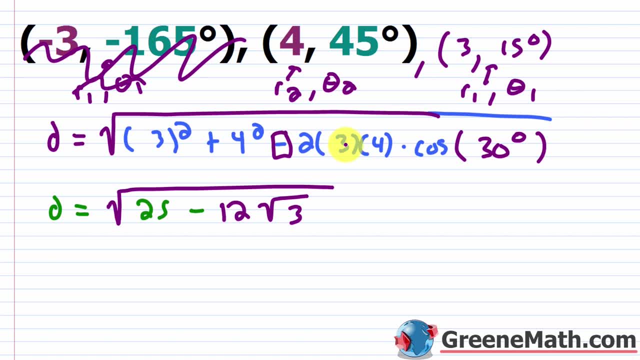 identity in a moment. that proves that this is basically going to work, right. So if you add 180 degrees to your angle, okay, it's going to change the cosine of that from negative to positive, Okay, Or from positive to negative. So, essentially, what I have here is nine plus. 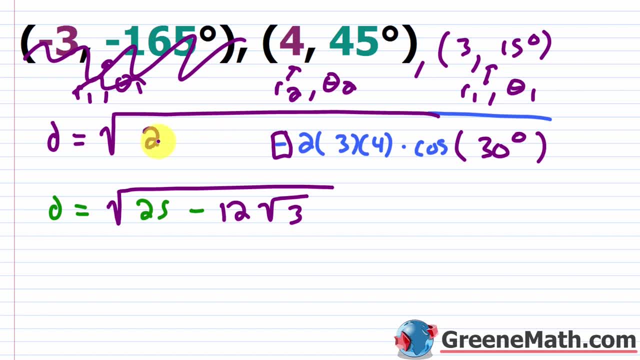 16, which is 25 again. So that part is the same, Okay. And then here we have: okay, we're going to do what we were doing before. Okay, We're going to remove the sin and we're going to remove the sine two times three, That's positive 60. If you add up plus negative two. 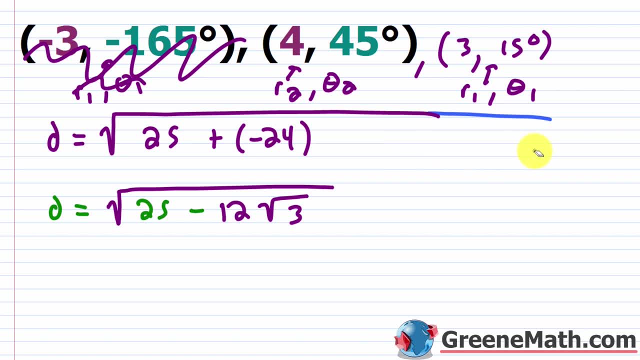 times three there, it's going to give you 25.. If we're going to multiply that by the cosine of 30 degrees, we know that this is going to be the square root of three over two, Okay, So from here this cancels with this, Again, it's negative times positive. 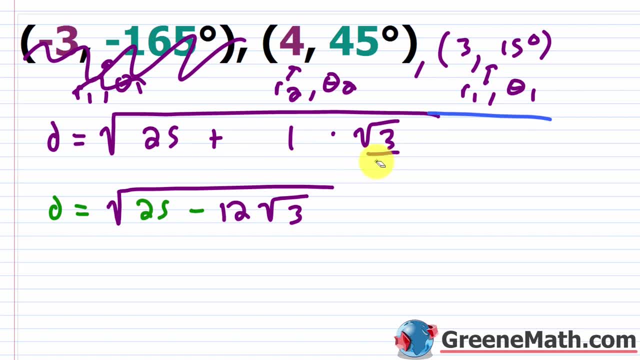 so it's still negative. So it's going to be negative 12.. So, negative 12.. Let me erase that and put negative 12 times the square root of three, So you see, you get the same answer either way. okay. So let's talk about why this works. Let's get rid of all of this Again. 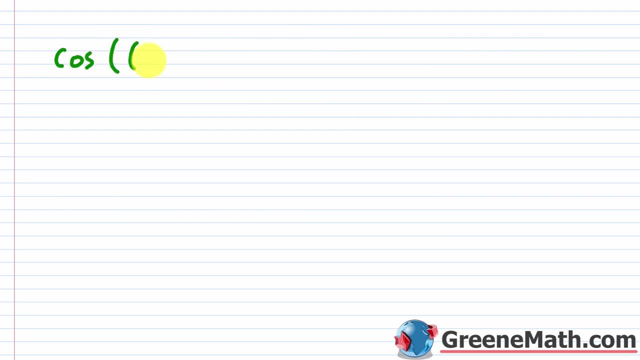 when I think about something like the cosine of some angle theta plus 180 degrees, this is going to be the negative of the cosine of theta. So you saw, with our example, we basically had a theta that was 30 degrees, right? If I added 180 degrees to that, I got 210 degrees and that's going to 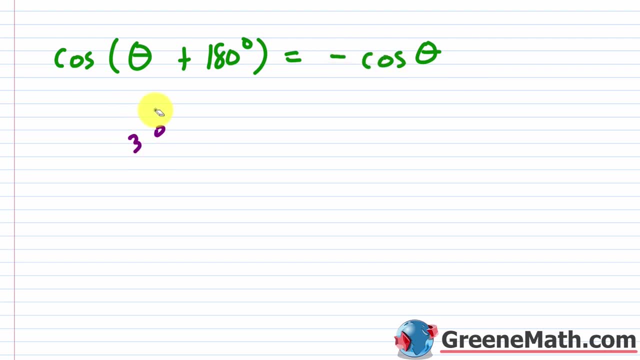 be the negative of the cosine of 30 degrees. okay, Again, you can prove this with the cosine sum identity. So if you wanted to do this, you could say that you had what The cosine of the first guy, theta, and then basically times the cosine of 180 degrees. Now you know this is negative one. 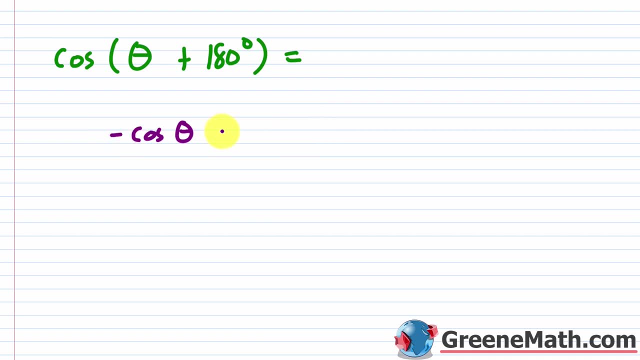 so you can just replace that, Just put a negative out in front and then you're going to go minus, right, Because it's always the opposite sign. So it's going to be sine of the first guy. so theta times the sine of 180 degrees. Now the sine of 180 degrees is zero, so you can get rid of this. 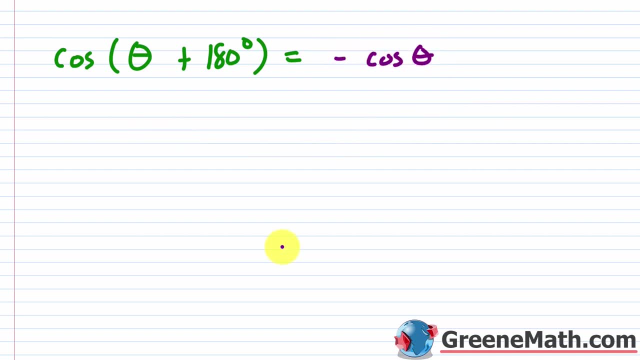 and you're just left with the negative of the cosine of the first guy. theta times the sine of 180 degrees. So it doesn't matter if you get a negative R value. If you change that over to a positive, then your angle is going to increase by 180 degrees. okay, So you're going to change the. 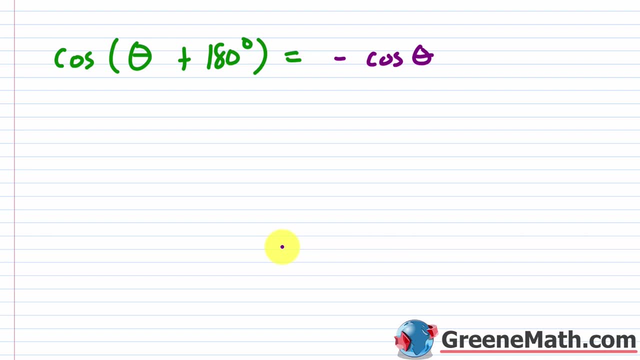 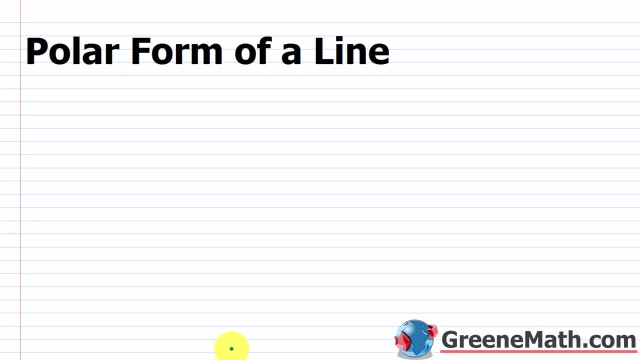 signs on the middle part, but then you're going to compensate for that, because your cosine value is going to change signs as well. so you're going to come back to the same answer. In this lesson we want to talk about the polar form of a line. All right, so we've spent a lot of time talking. 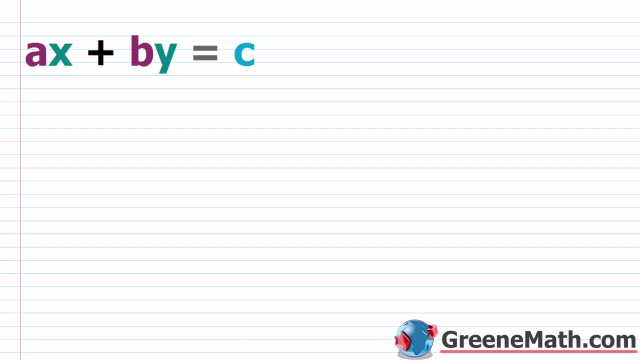 about the polar coordinate system and also how to convert rectangular coordinates to polar coordinates and then take those polar coordinates and plot them on the polar grid. What we're going to do now is take the next step and talk about polar equations. okay, So we're 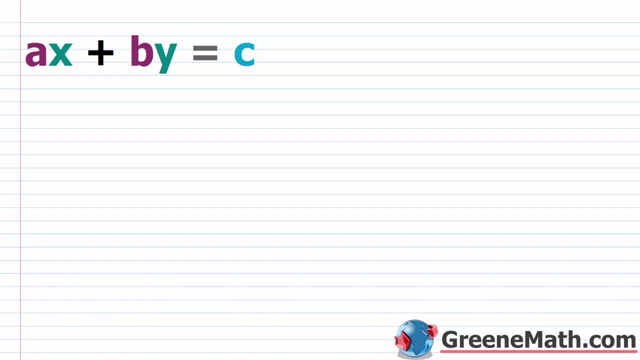 going to need to know how to convert between the rectangular form and the polar form, and we're also going to need to know how to graph these equations on the polar grid. So today we're going to start out with something very simple. It's the polar form of a line and basically, 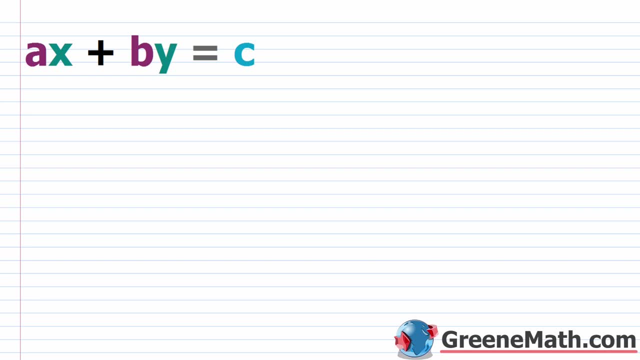 graphing them and converting them back and forth between the rectangular form and the polar grid. Okay, so, basically, what you need to know is if you're going from your rectangular form to your polar form. it's very, very simple. You're going to use a relationship that we've 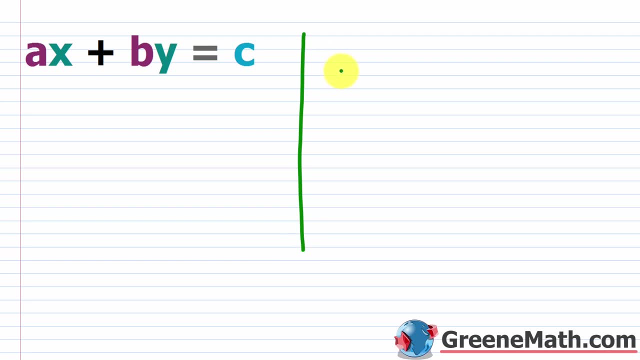 talked about many times, and that's basically that the sine of theta, going back to the original definition, is y over r. right, You could say opposite over hypotenuse. and the cosine of theta is equal to x over r, the adjacent over the hypotenuse. 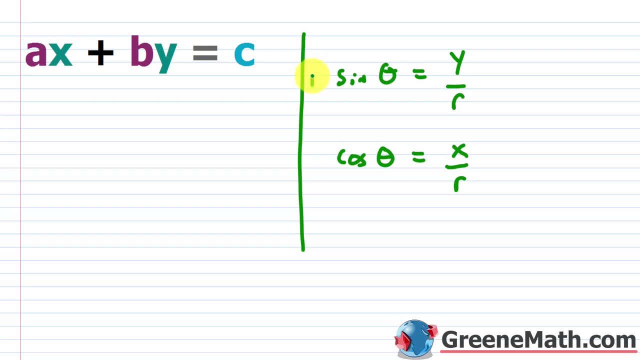 What we're going to do in each case is multiply both sides by r. So I'll say: this is r times sine of theta. multiply this by r, and that would cancel. So you've solved this for y here. Same thing over here. multiply this side by r and this side by r. this would cancel over here. 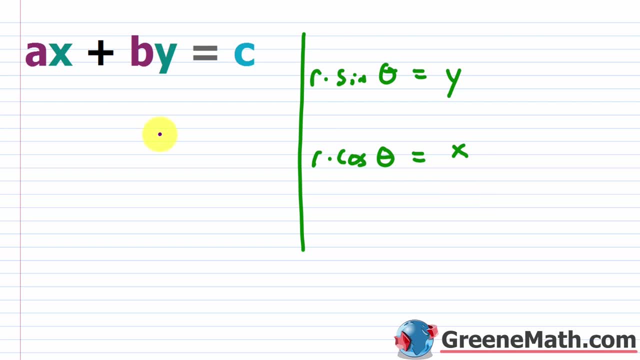 And what you end up with is a relationship you're going to use to convert this. okay, So I'm going to take this right here: this r times sine of theta and I'm going to plug it in for y. And then I'm going to take this right here: this r times cosine of theta and I'm going to plug it. 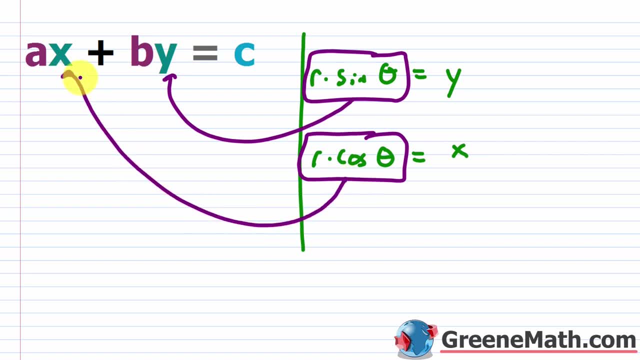 in for x. That's all you need to do. Depending on your teacher, they may have you work with some generic form. So this is the standard form of the line. You also have the slope-intercept form. the y equals mx plus b, If you're working. 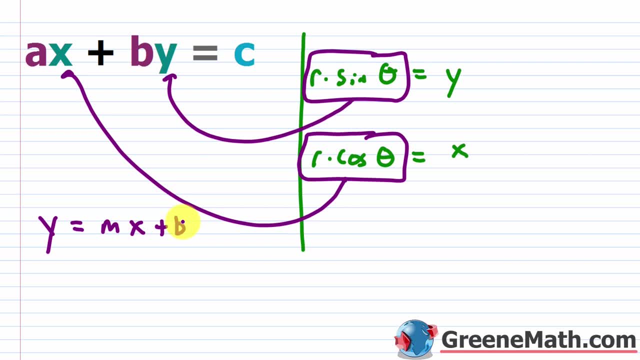 with this a lot. you may need to convert it over generically, okay, And then you could just plug in for your a, b and c, okay, Or in this case, you would just be plugging in for your m and your. 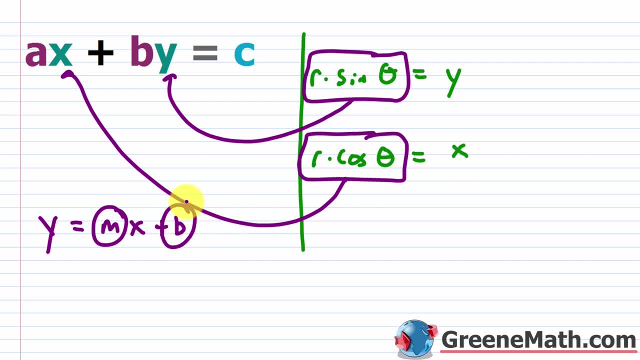 b. okay, But it just depends on what you want to do. Let me just go ahead. I'm going to solve this generically and then, on the first example, what we'll do is we're going to plug in for y and then 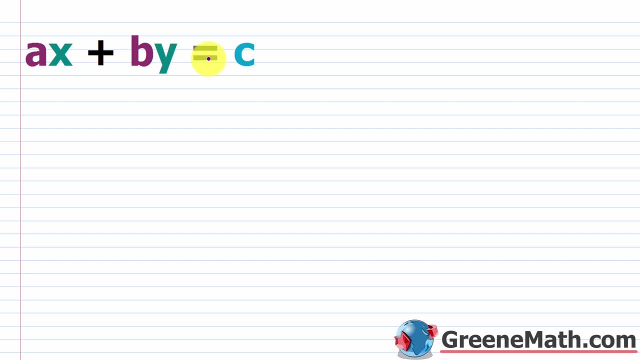 we'll just plug it in that way and then I'll also plug it in the other way. I'll show you it's the same thing, okay? So let's just go ahead and plug in r times cosine of theta here and then r. 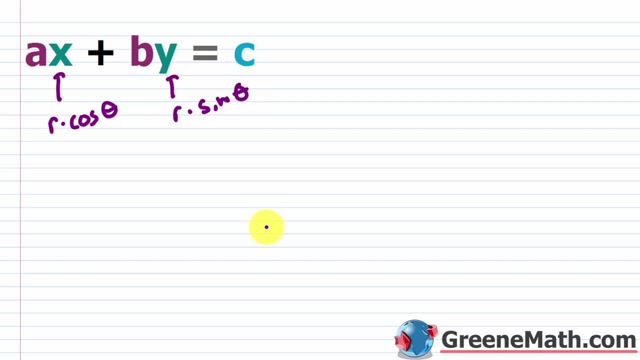 times the sine of theta here. okay. So what would we have? You would have a multiplied by r times the cosine of theta, plus you would have your b times your r times your sine of theta, okay, And this just equals c. Now, the idea here is that you're going to factor out the r, okay, And then 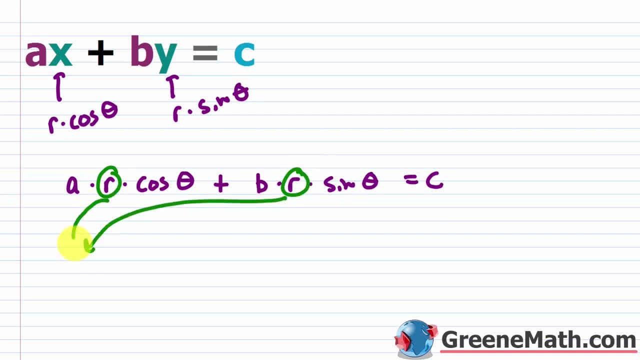 to solve for r. So if I pulled that guy out, okay, if I pulled that guy out, I would have r times the quantity What's left Your a times your cosine of theta. so a times cosine of theta plus your b. 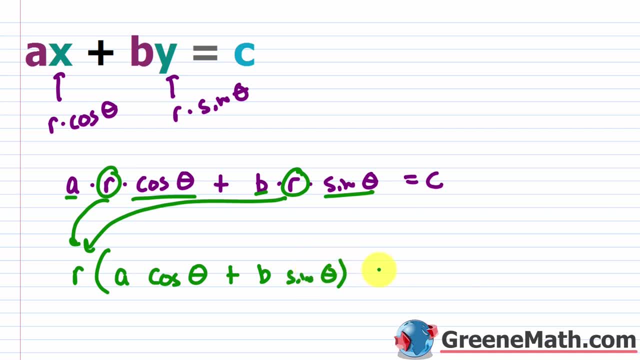 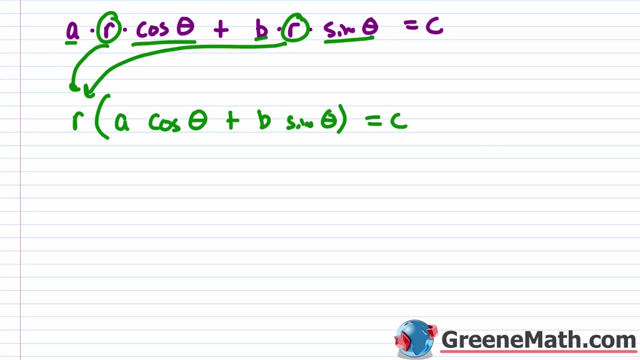 times your sine of theta, So your b times your sine of theta, and this is equal to c. okay, So let's stop for a minute. Let's scroll down, get a little bit of room going. How can we solve this for r? Remember, this whole thing is a quantity and it is multiplying by r. okay, So what I can. 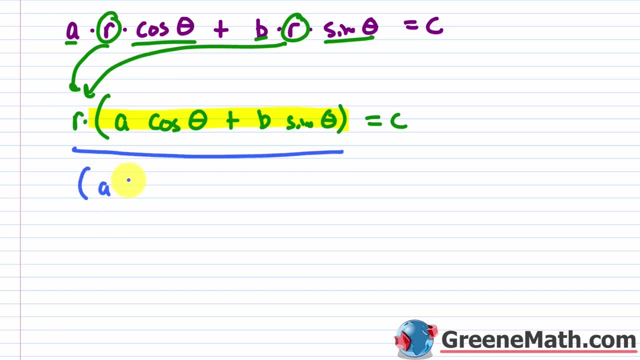 do is just divide Both sides by this quantity: this a times the cosine of theta, plus b times the sine of theta. okay, Perfectly legal. And so what's going to happen is this is going to cancel with this. That will be one. So you have r by itself and it's equal to and over here, let me scooch this down. 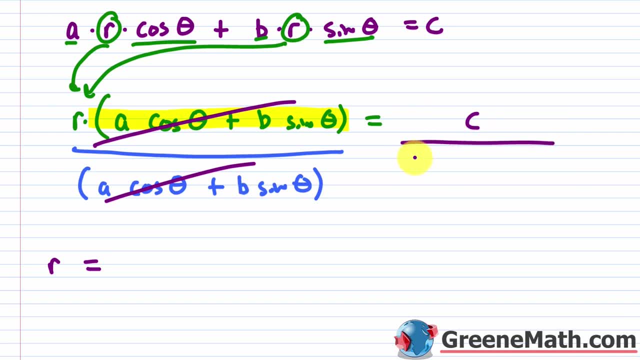 a little bit so this looks a little bit better. I'm going to divide this by the same thing. So a times the cosine of theta plus b times the sine of theta. okay, So r equals. you have your c, which is your constant, from the ax plus by equals c. 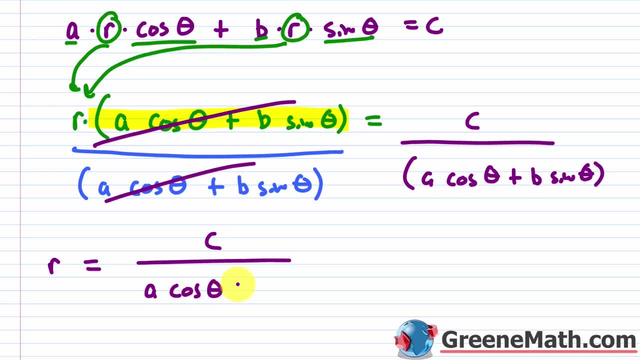 Over your a times your cosine of theta plus your b times your sine of theta, where the a is the coefficient from x and the b is the coefficient for y. Now you could do a similar process with the y equals mx plus b. Get yourself a general formula for that. It's up to you in terms of how. 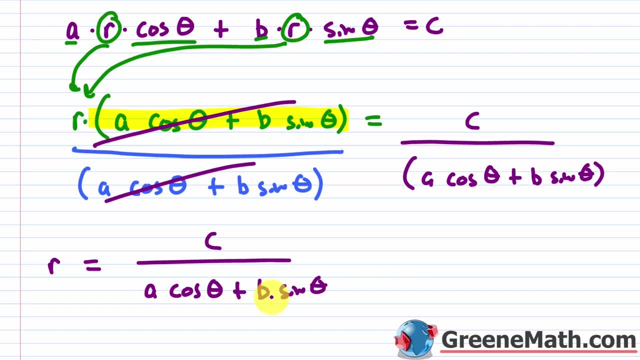 many of these problems you're going to have to solve, and whether it's worth or not to use a general formula or just plug in each time, okay. But what I want to say is, if you're going to use this formula, make sure that your line. 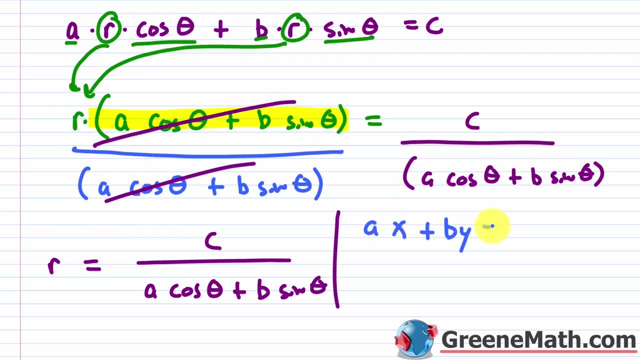 is in the format of ax plus by equals c. It must be in this format. to use this formula, okay, It's very, very important because a lot of times you get the slope intercept form or something else given to you okay, And people start plugging things in and they get the wrong answer. So 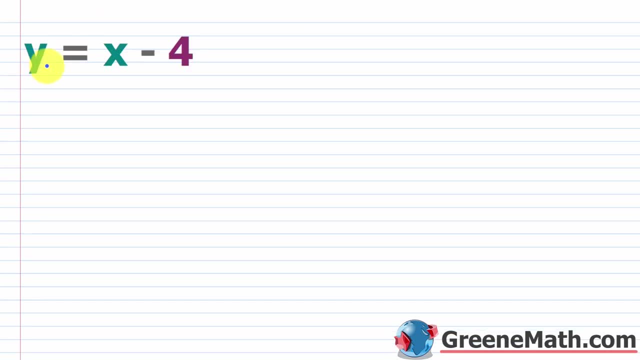 let's go ahead and just look at a simple example. So here we have y equals x minus 4, okay, This is in slope intercept form. So this follows: the y equals m, the slope times, x plus b, the y intercept. okay, So we know this. 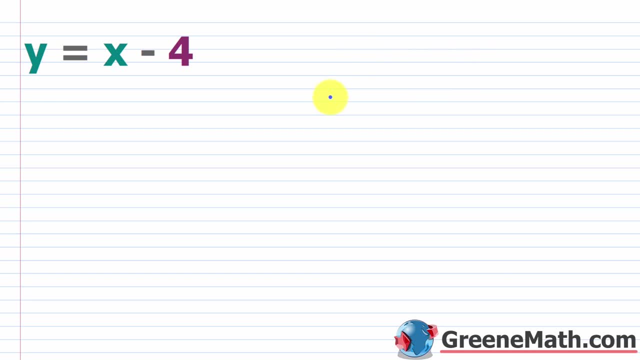 We want to convert this to standard form so we can use that little formula. Then what we would do is we would subtract x away from each side. okay, So I would say that I have negative x plus y is equal to negative 4.. Now for myself, I prefer the high school definition of the standard form of the. 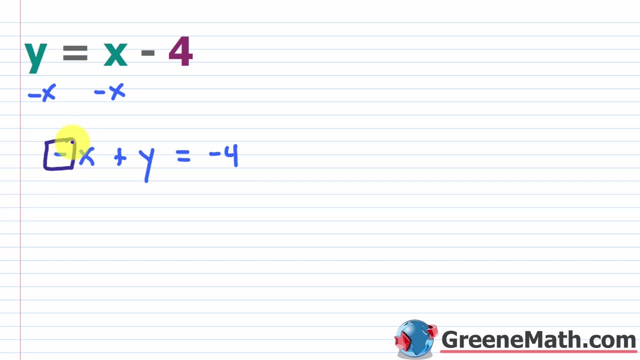 equation of a line, and so I want the coefficient here for x to be positive, and to do that, I'm just going to multiply everything by negative 1.. So this would be: x minus y is equal to 4,. okay, It just changes the sign of every term. 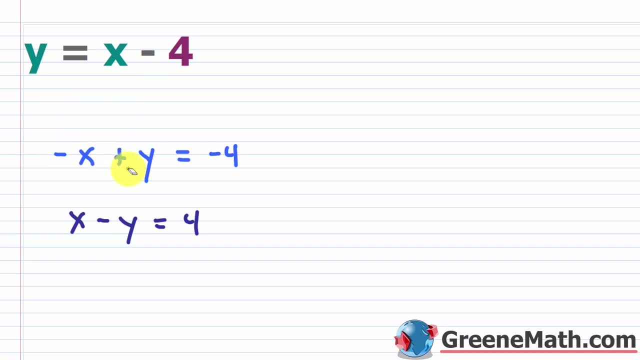 When you multiply both sides by negative 1,. okay, So let me actually erase this and this. okay, And at this point, basically, you can use your formula. You know that the coefficient for x is a 1,, the coefficient for y is a negative 1, and your constant is a 4.. So, in other words, the a value is: 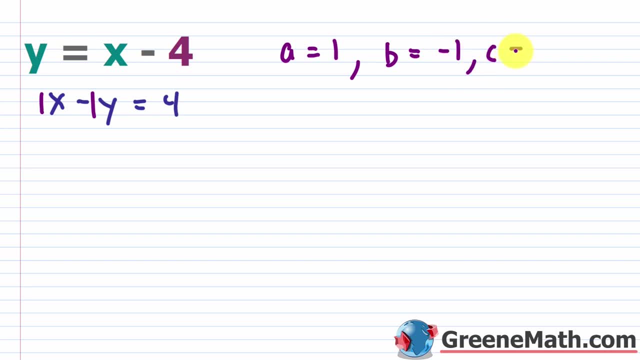 1, the b value is negative 1, and the c value is positive 4.. So remember, r is equal to. you have your c over, you have your a times cosine of theta plus your b times cosine of theta and you have your. 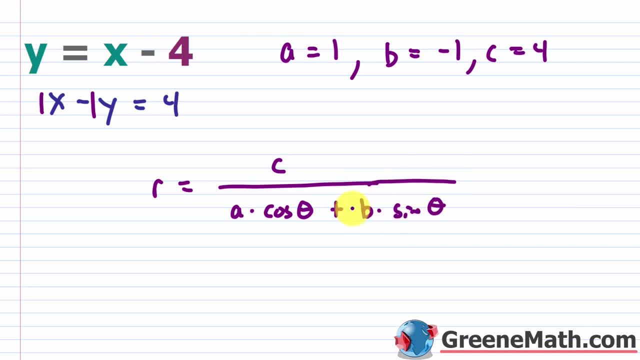 b times your sine of theta. okay, If you do this a few times, you will memorize it. Now, what I'm going to do is just plug in. So, instead of c, I have 4.. Instead of a, I have 1, so you can just get. 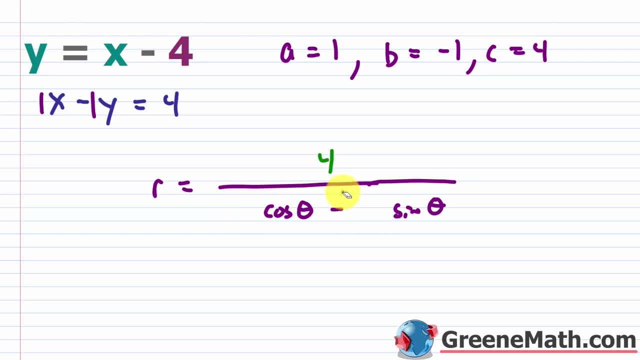 rid of that, And instead of b I have negative 1, so I can just change this to a minus And that's all it is. So r equals 4 over the cosine of theta minus the sine of theta. okay, Now you might be. 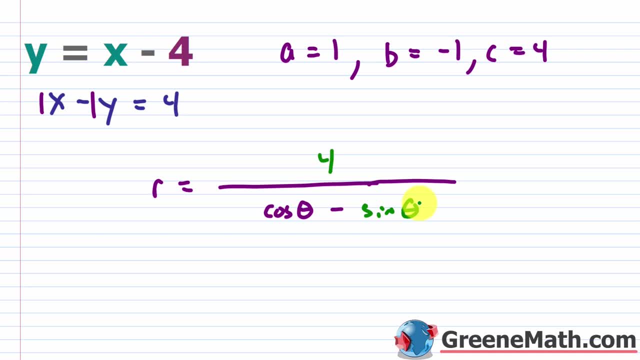 thinking: how in the world are we going to graph something like this? And I'll show you that in a moment, But really quickly, I just want to show you if you had done this data you would have the other way that you would get the same answer right. So, basically, if I plugged in r times cosine, 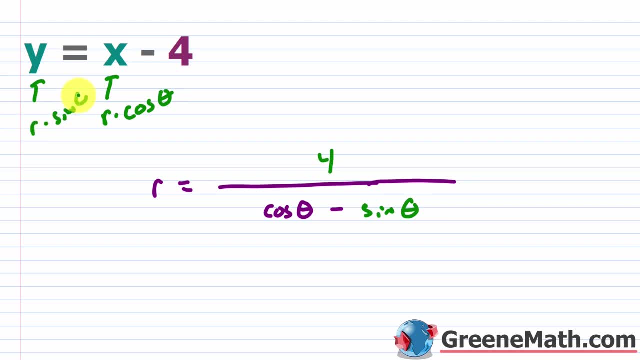 of theta there and I plugged in r times the sine of theta there, I could achieve this same result. okay, So what I could do is say I have r times sine of theta, And then what I'm going to do is say I'm going to subtract this right here, away from each side. So I'll say: minus r times cosine. 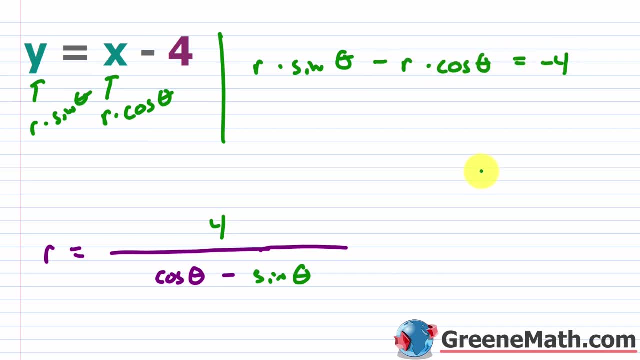 of theta, and this is going to be equal to negative 4,. okay, And from here, what I'm going to do is I'm going to factor the r out, So I'll say r times the quantity sine of theta, and then I'll say minus the cosine of theta, and this will be equal to negative 4,. 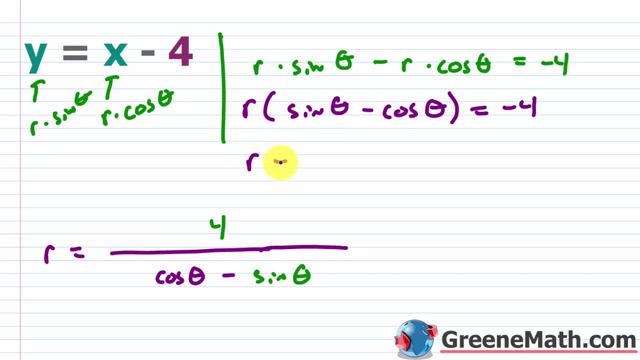 okay, And then I'm going to divide both sides by this, so that r is equal to you'll have negative 4 over. I'm going to go ahead and say I'm going to put negative cosine of theta first and then. 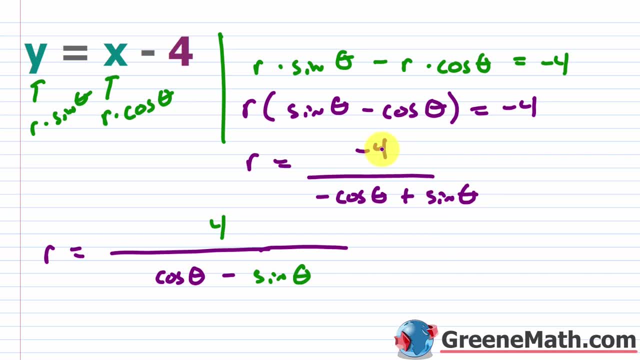 plus the sine of theta right. So the only difference between this and this is the sine, And of course, what you could do here is you could multiply the numerator and denominator by negative 1,. okay, That's perfectly legal, because that's a complex. 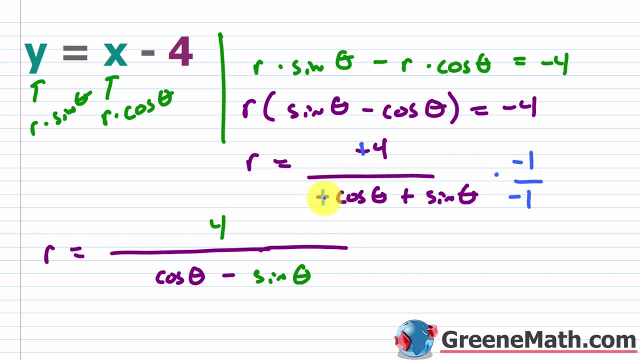 form of 1.. So this would become positive. this would become positive and this would become negative, And essentially, what would happen here is your two forms would match up completely right. r equals 4 over cosine theta minus sine of theta in each case. Okay, so let's erase all of. 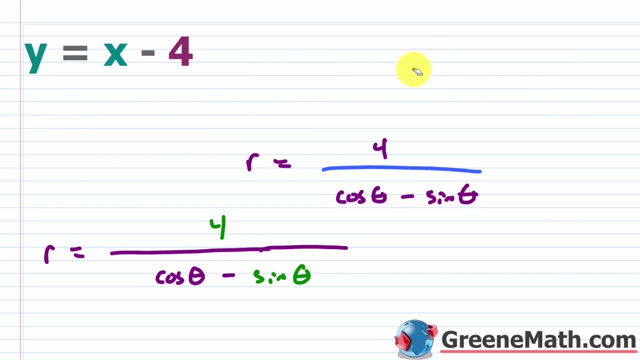 this and let's talk about graphing now. So graphing a polar equation is probably one of the best ways to graph, and with a line it's a little bit more challenging. Lines are a lot easier to graph on the rectangular coordinate plane. To see this really quickly, let's think about: y equals x. 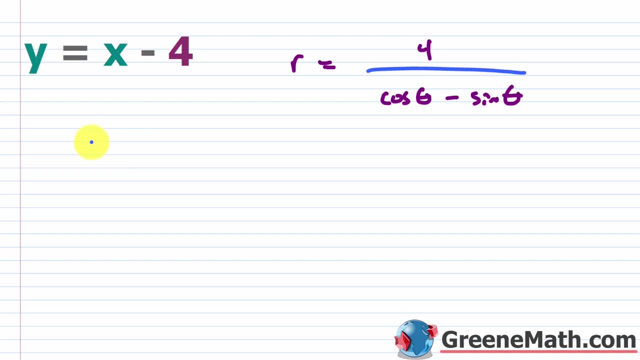 minus 4 on the rectangular coordinate plane. We know that the y-intercept, the y-intercept is going to be at 0 comma negative 4, and m, the slope is equal to 1,. right The coefficient for x. 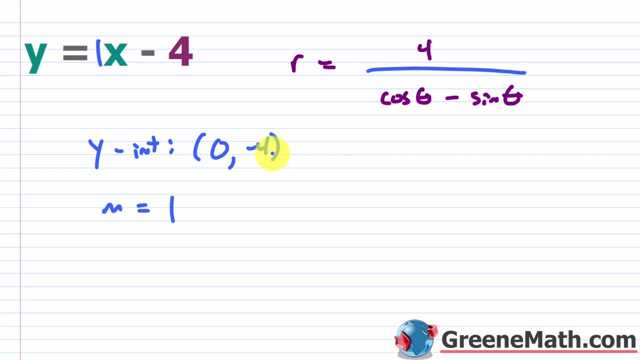 So essentially I could plot 0 comma negative 4, and then just use my slope of 1 to get additional points. So if I come here I can see that I just dropped the slope of 1, and I can see that I just 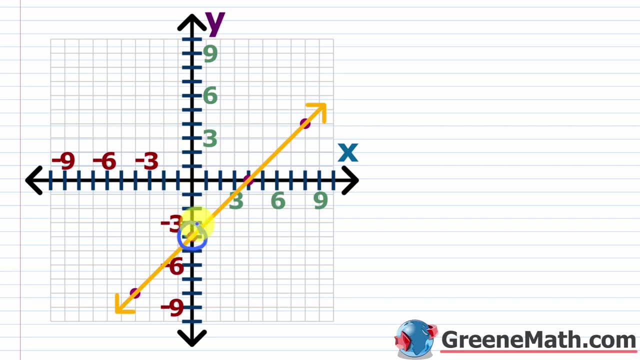 dropped the slope of 1, and I can see that I just dropped the slope of 1, and I can see that I just dropped down to 0 comma negative 4.. That's right there, And then I can use my slope So up 1 to the right. 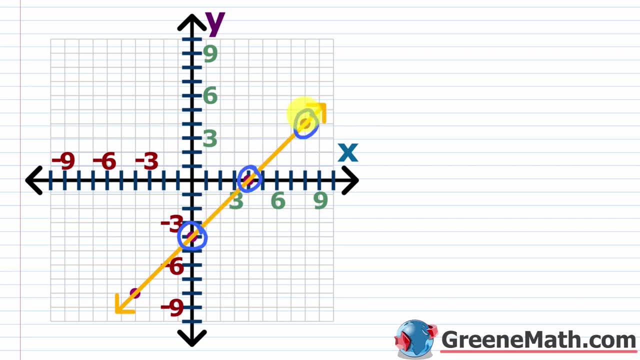 one up, 1 to the right one, you know, so on and so forth. I could generate this point and this point and this point, As many points as you need. You only need two points to get a line. A lot of. 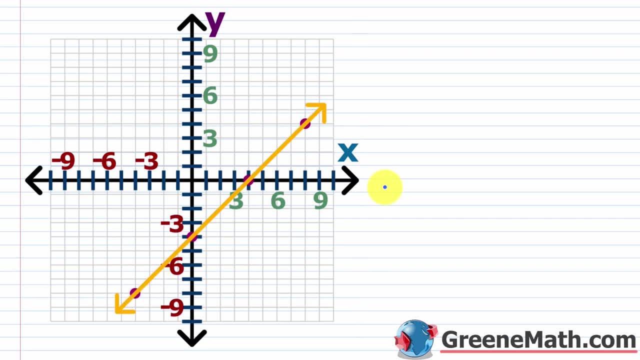 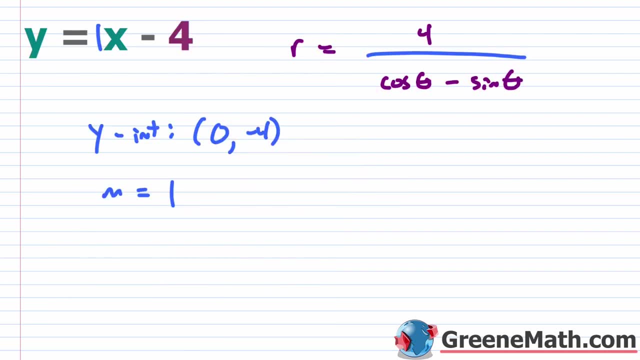 times people like three to get a check, but you only need two. Now let's say that I wanted to graph that equation in polar form on the polar grid. What could we do? Well, you can go back to your original strategy of making a table of values. So we would go back, just make a little. 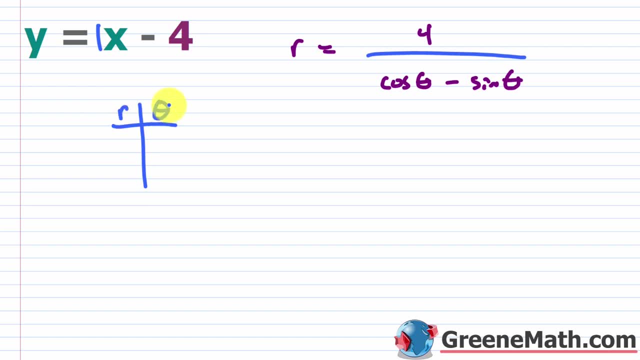 table and say, okay, I have my r value and my theta value And I like to plug in values for theta- okay, and then get a value for r. So what I'm going to do here is I already know that the 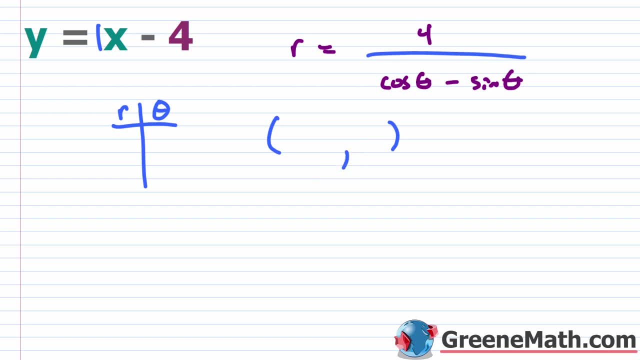 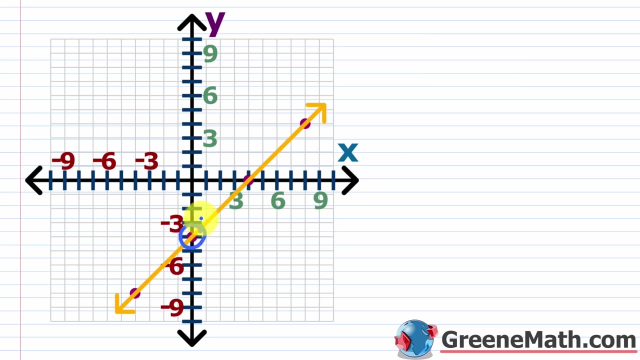 y-intercept occurs at 0 comma negative 4.. That's pretty easy to convert over. So this point right here. you can use the traditional method to convert it over. That's up to you. But what I'm going to do is just think about the fact that, okay, if I'm starting here, at the origin, I need 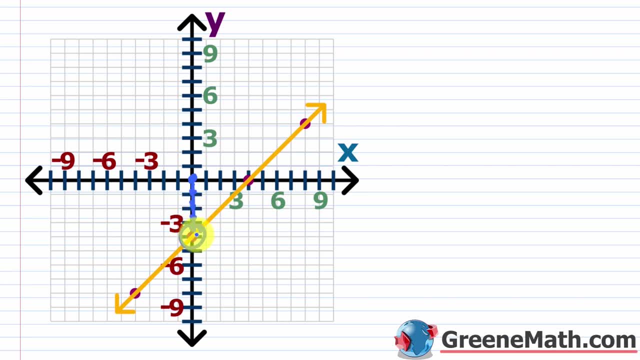 to travel 1,, 2,, 3, 4 units together. So I'm going to do that. I'm going to do that, I'm going to get there, okay, And essentially the angle here is going to be 270 degrees. I know the r value is. 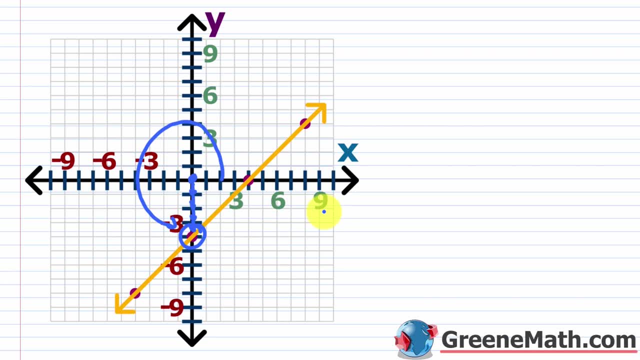 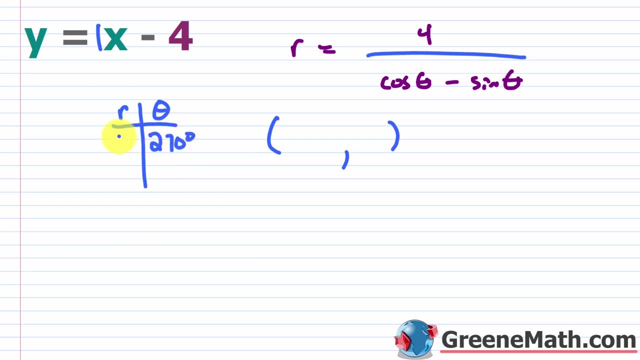 4,. okay, not negative 4,, but 4.. And the angle is 270 degrees. So if I come back, I can say that a theta value of 270 degrees would give me an r value of 4. And you can check this out If you. 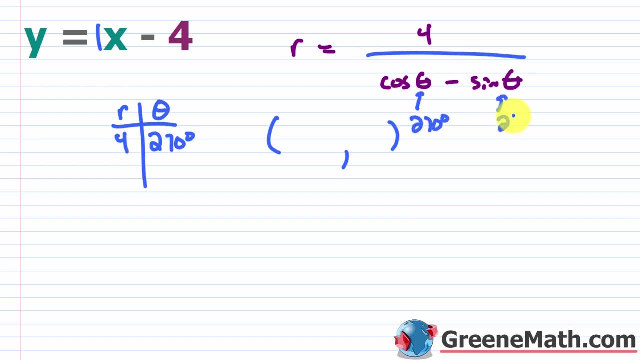 plug in a 270 degrees there and also there. what would you get? Well, the cosine of 270 degrees is 0, okay. So essentially you would have 4 over. You would have 0 minus. The sine of 270 degrees is negative 1, minus. the negative 1 is 1, okay. 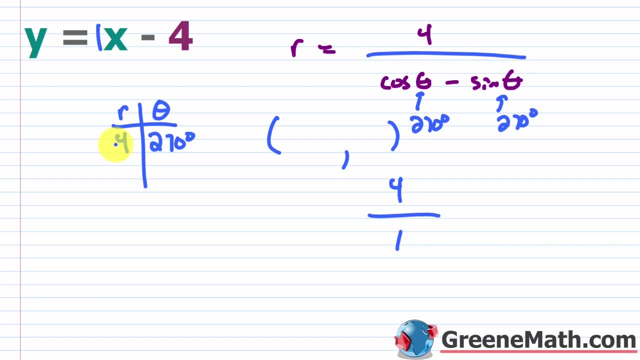 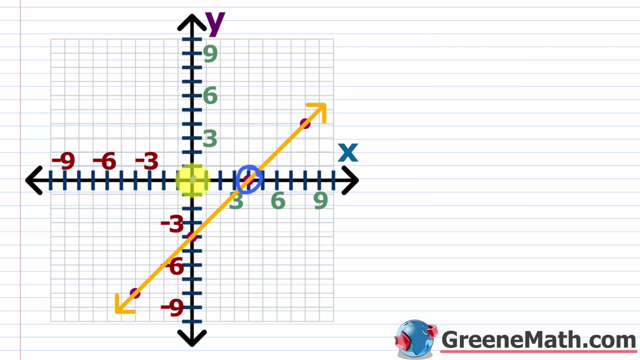 So essentially you would have 4 there, right? So you would get 4, 270 degrees as one of your points, okay. Then the other one. if you think about your x-intercept here, well again you can go back to your graph that this guy right here is 4, 0, okay, So essentially from the origin. 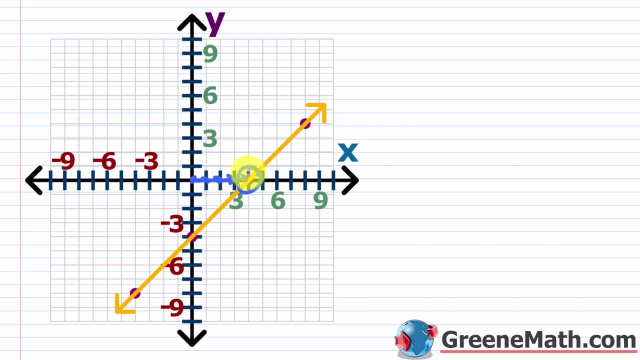 I have moved 1,, 2,, 3,, 4 units to the right, So the r value is going to be 4, okay, But the angle here is going to be 0 degrees right, Because I'm on the positive x-axis. 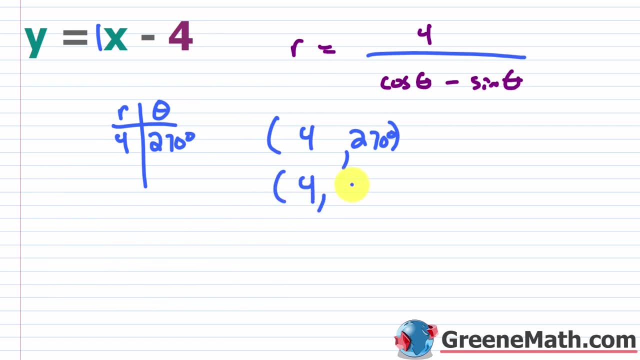 So, if I go back, that point would be 4, 0 degrees. okay, Again, you can plug this in. Plug in a 0 degrees here and a 0 degrees here. You would have 4 over The cosine of 0 degrees. 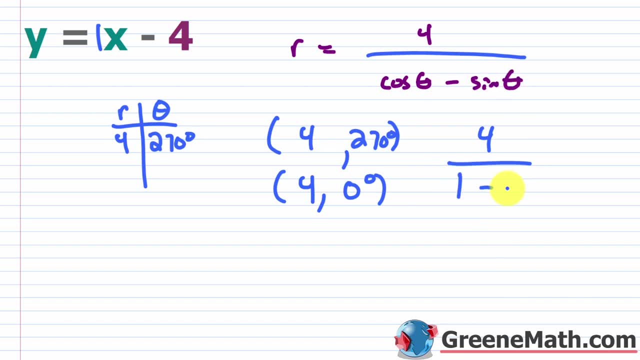 is going to be 1, and then minus the sine of 0 degrees is going to be 0. So this would be 4 over 1, which is 4, okay, So that's another point. So 4, 0 degrees, All right. so now that we have these, 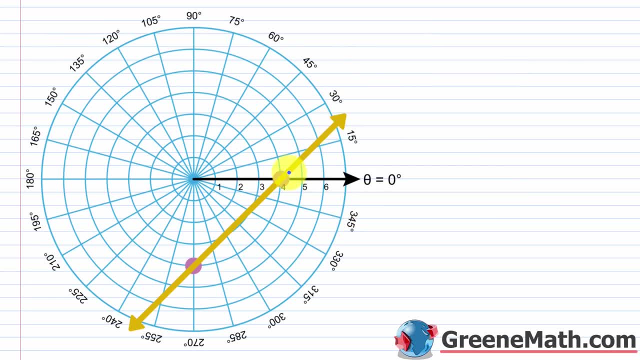 two points. we're going to go back to our equation. We're going to go back to our equation. We're ready to sketch our graph. So again, our two points. we have the 4, 0 degrees. That's going. 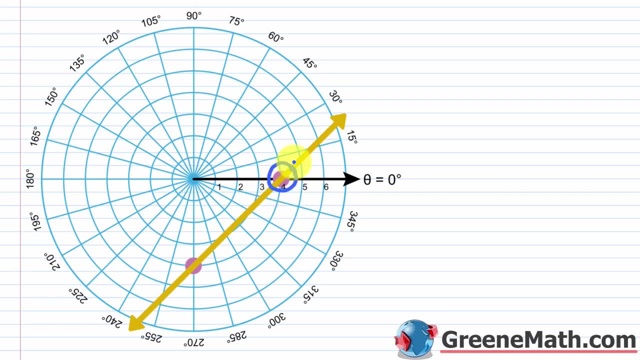 to be right here And the other one is going to be 4, 270 degrees. So I'm going to be swinging around to right here. So that's right there, And then, basically, once you have those two points, that gives you a line So you can sketch that guy and you are done. Okay, let's look at another. 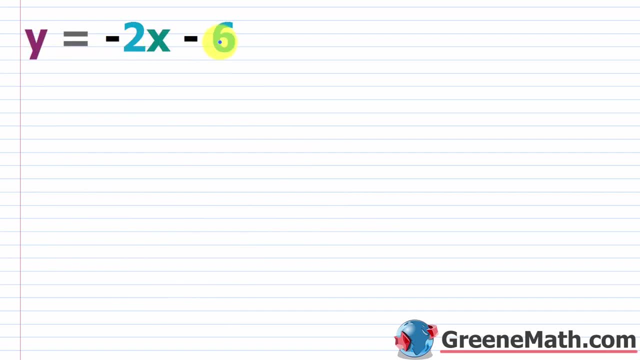 example. So here we have: y equals negative 2x minus 6.. Again, you can put this in standard form and use your formula. You can plug in for x and y whatever you want. So you can plug in for y whatever you want to do. I'm just going to use the formula. So I'm going to add 2x to both sides. 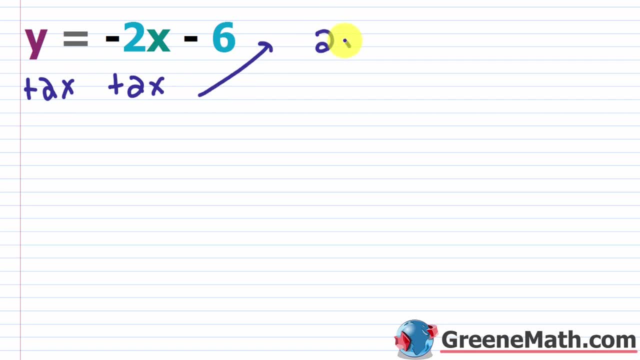 of the equation, And I'll go ahead and say that this is 2x plus y, is equal to negative 6.. So my value for a is 2.. It's a coefficient for x. My value for b is 1.. And let me put that in visibly. 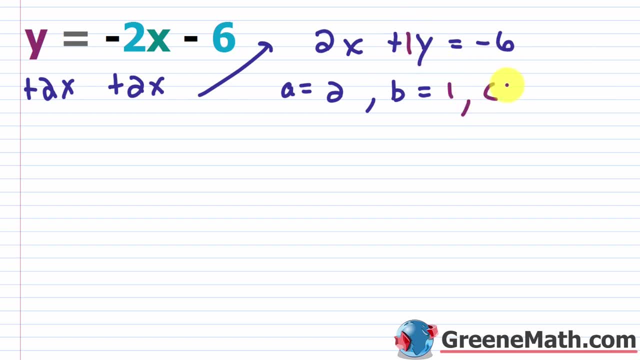 okay, That's going to be my coefficient for y And then my value for c. my constant is negative, 6.. Okay, so now I'm just going to plug into the formula. I'll say that r is equal to. you're going to have your c value, which is: 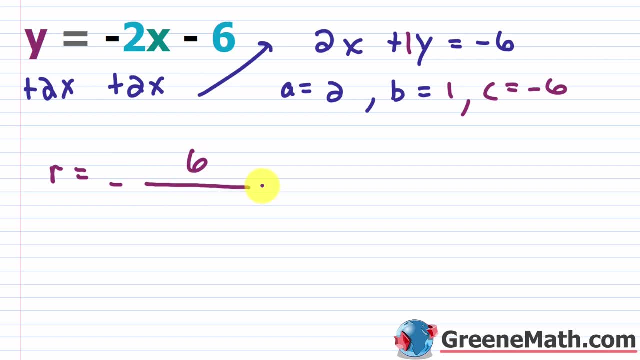 6.. Let me put a negative out in front. I'll put the 6 out up here, And then over you have a which is 2, times the cosine of theta, And then plus you're going to have your b value, which. 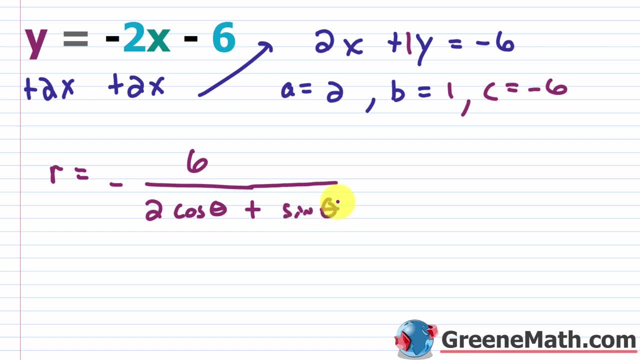 is 1, so don't write anything. times the sine of theta. Okay, so that's all it is. So this is our equation. You can see that using that formula is pretty quick And, essentially, if I want to graph this again, the simplest way for me to do this is to think about this on the rectangular plane. 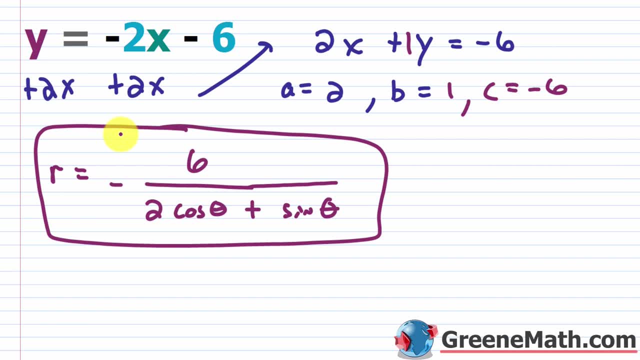 If I can get the x and the y intercept, that's going to give me two points that I can really quickly convert over to polar form, and I'm done okay. In some cases you won't be able to do that. I'll give you an example of that later on. So here, what I'm going to do is I'm going to 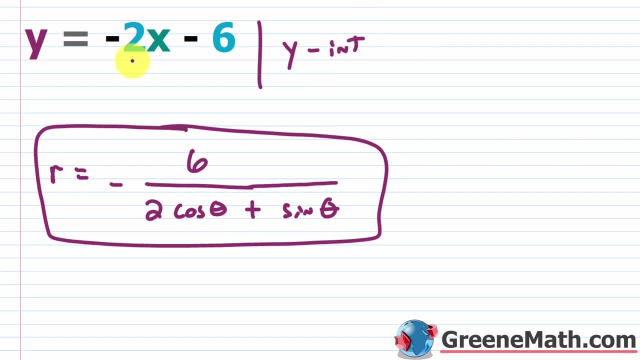 say, okay, well, the y intercept. the y intercept- since this is in slope intercept form, I know- is at 0, negative 6.. So think about this: If I was at the origin, I would be going down 1,, 2,, 3,, 4,, 5,. 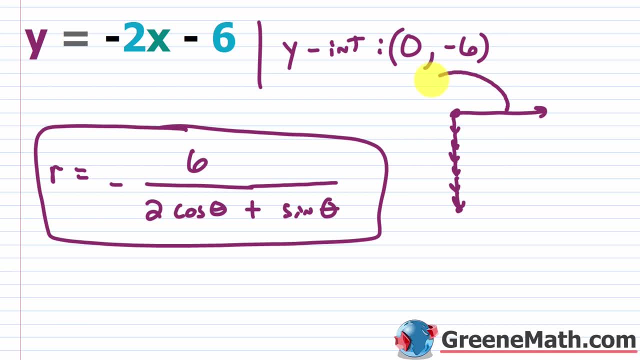 6 units to get there. okay, And from the positive x-axis I'm swinging around 270 degrees. And again, if you're not comfortable with what I'm doing, just take the normal steps to convert this that we talked about over the course of the last two lessons. okay, Then the other guy here. 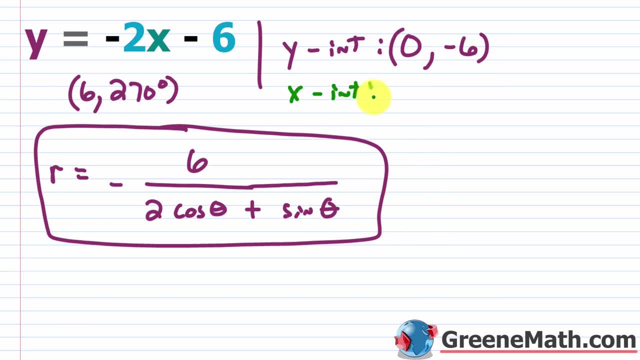 the x-intercept. the x-intercept, if we think about that. well, if I plugged in a 0 there, I would have. basically: 0 is equal to negative 2x minus 6. Add 2x to both sides, so 2x is equal to. 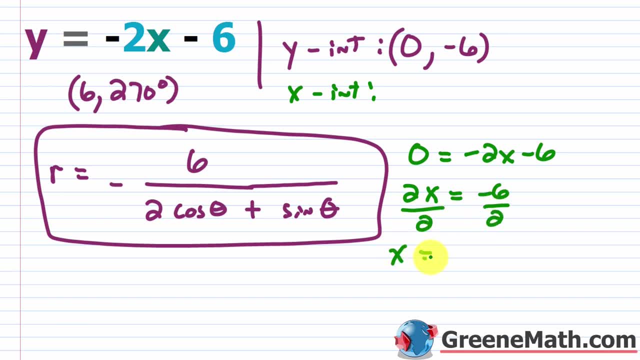 negative 6.. Divide both sides by 2, you get. x is equal to negative 3,. okay, So this would be negative 3, 0.. So in polar, what would that be? Well, negative 3,. if I start right here, let's say we're going to go 1,, 2,, 3 units to the left. 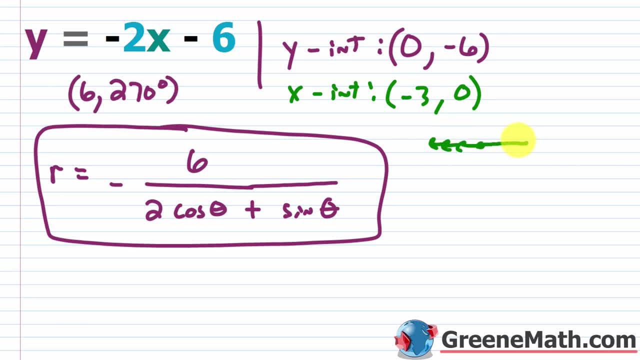 okay, Don't worry about it being negative. it's 3 units to the left And the angle with the positive x-axis we're going to come around 180 degrees. okay, So this guy is going to be- let me, kind of. 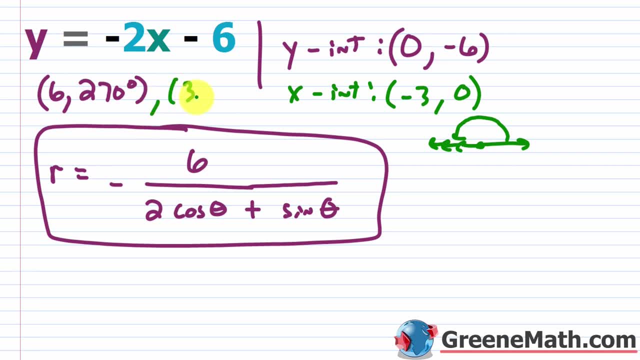 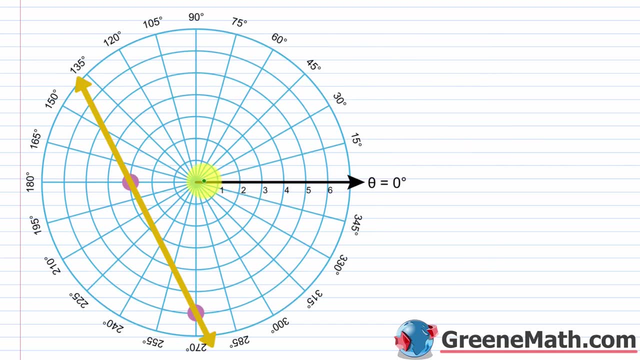 scooch this down a little bit. this guy is going to be 3, 180 degrees, okay, So that's going to be my two points in polar. So if I come over here again, I go out to a circle with a radius of 3,. 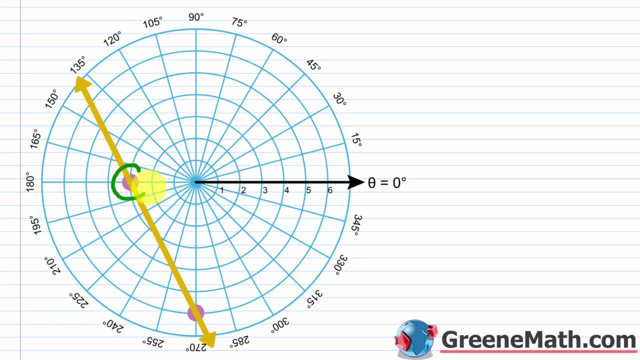 I'm going to swing around to 180 degree angle. so there's that point there. Then, for the other guy, I'm going to go out to a circle with a radius of 6, and I'm going to swing around here to an angle. 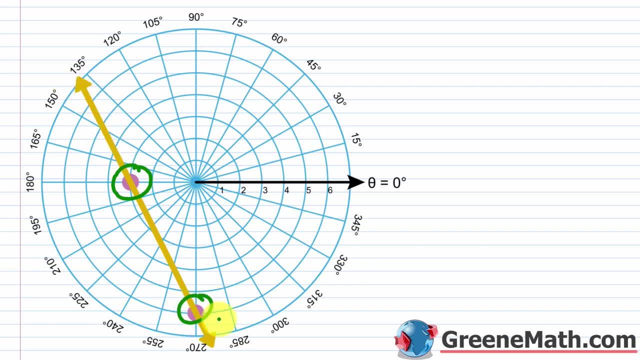 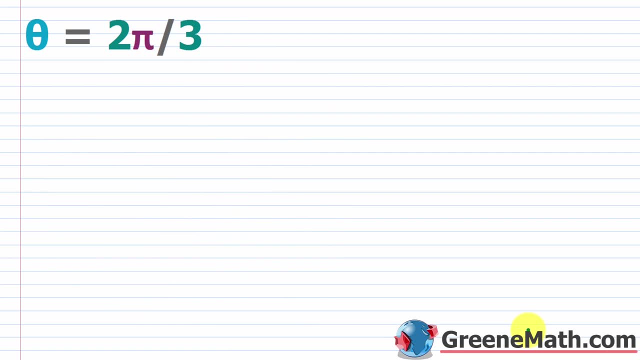 of 270 degrees. okay, Then you can just sketch a line through those two points. Okay, let's now talk about the harder scenario. This is where we're going from the polar form to the rectangular form. You need to understand a few relationships. The first one is that the tangent of theta is equal to. 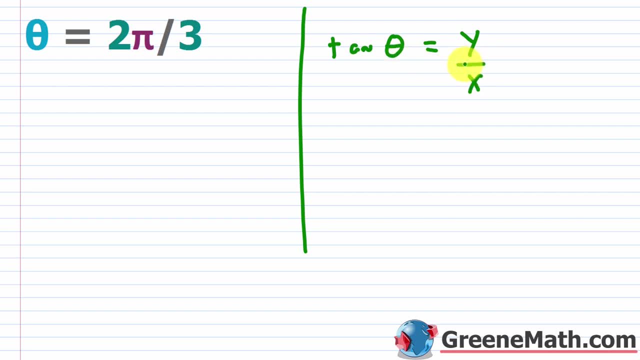 y over x. Just going back to that definition. you're going to need this a lot. Also, you're going to need to know that r is equal to the square root of x squared plus y squared. Again, we've talked about that a lot and we'll see how to use these as we go forward. okay, But right now, 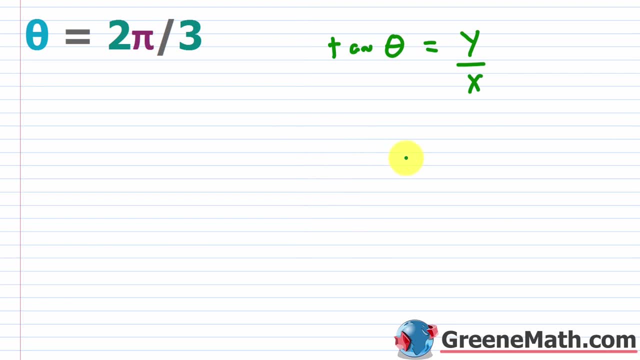 I'm just going to use this relationship here, okay, And so I have that theta is equal to 2 pi over 3.. Now, because my polar grid is written in degrees, I'm going to change this and say theta is equal to 120 degrees, Okay. 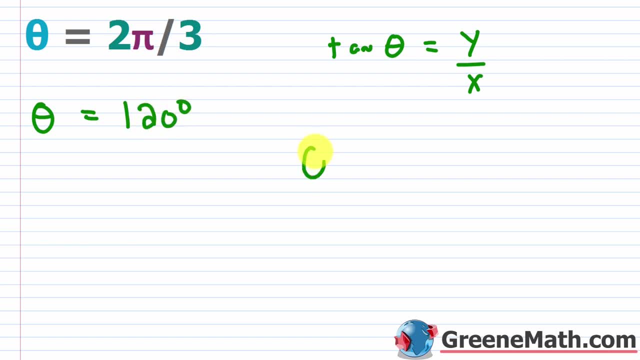 I'm just going to convert that over. And essentially, when you see something that's theta is equal to k, this is a line that passes through the origin. okay, We're thinking about it that way. Now, how can I convert this over? Well, to convert it over, what I would do is I would 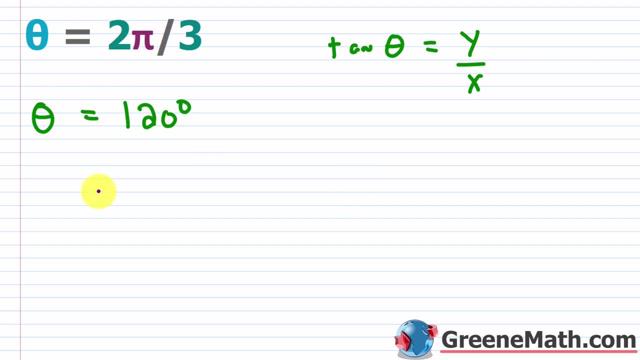 first take the tangent of each side. okay. So if I take the tangent of each side I would have: the tangent of theta is equal to the tangent of y over x squared. So if I take the tangent of each side, I would have the tangent of 1 over r squared. So if I give that a shot, I would see that it has. 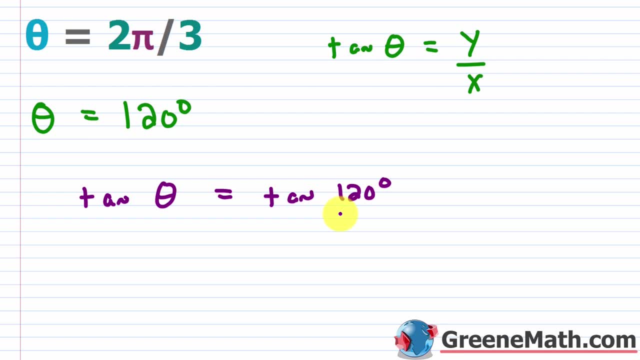 the tangent of 120 degrees. Okay, Now pause the video and think for a minute about how you can get this into rectangular form. How can I get this into an equation with x and y? Now, if you gave that a shot first, I would say: Okay, what is the tangent of 120 degrees? Well, it's the negative of 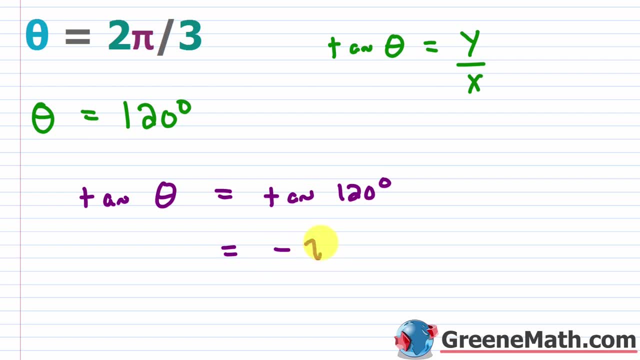 the square root of 3.. So let's erase this, or actually, let me keep this in line And let me actually keep that step there in case people get confused. So the negative of the square root of 3.. here you're going to replace that with y over x, because the tangent of theta is equal to, or the 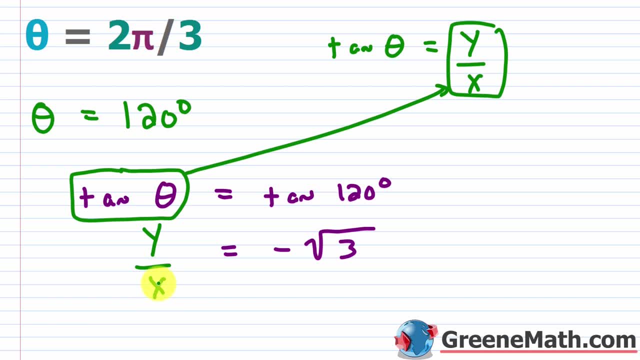 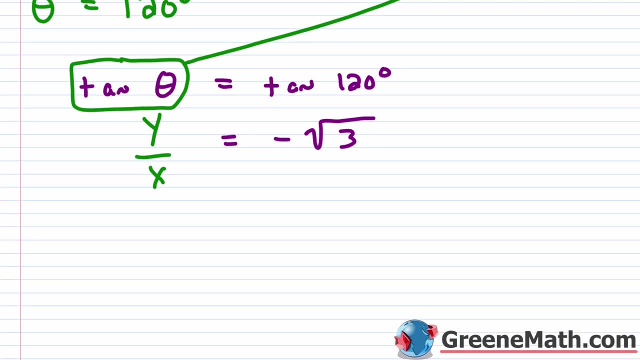 same as y over x. So I'll say y over x is equal to the negative of the square root of 3.. So once you realize that, it's pretty easy from here. All I really need to do is multiply both sides by x. 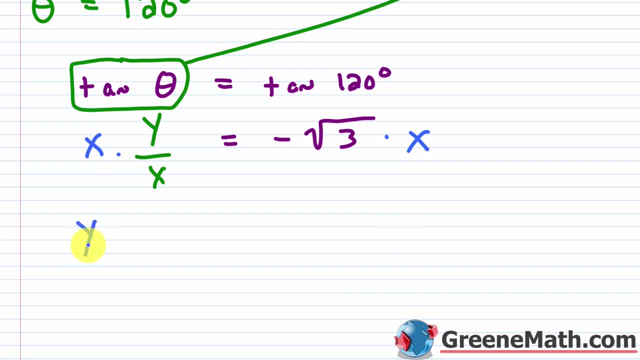 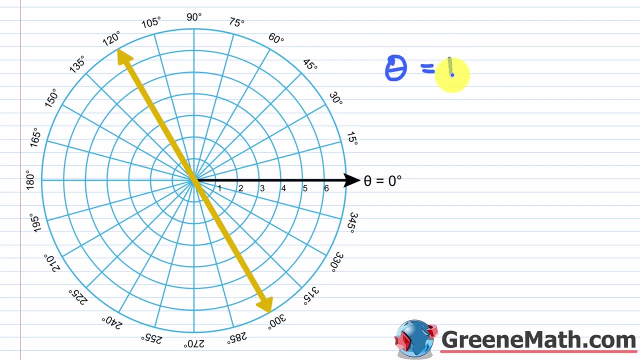 So multiply this side by x and multiply this side by x And I'll say y is equal to, I'll say, the negative of x times the square root of 3.. So this is the rectangular form of that equation. Now, if we think about graphing this again, if I had something that was, theta is equal to 120 degrees. 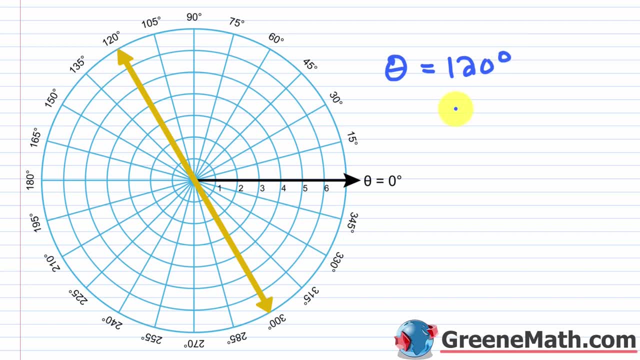 and you stop for a minute and think about that. you think about the fact that there is no r value given. So it means that no matter what the r value, whether it's positive, we know we can have negatives, that basically I'm going to be on 120 degree angle. So if I think about starting at the 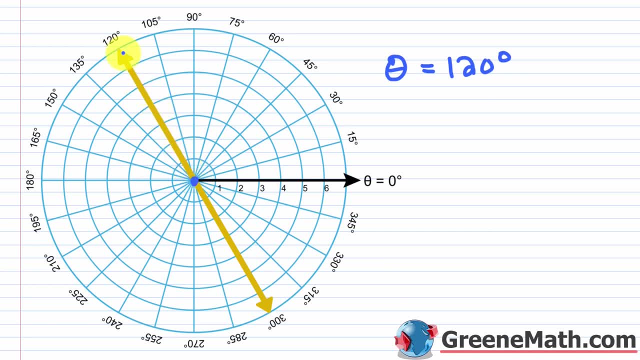 pole. here the origin. if I'm walking forward, I'm going to be on this 120 degree angle here. Remember how if you have a negative r value, you're going to be on a negative r value, You're walking backwards. So again, I would find 120 degrees and I would walk backwards. 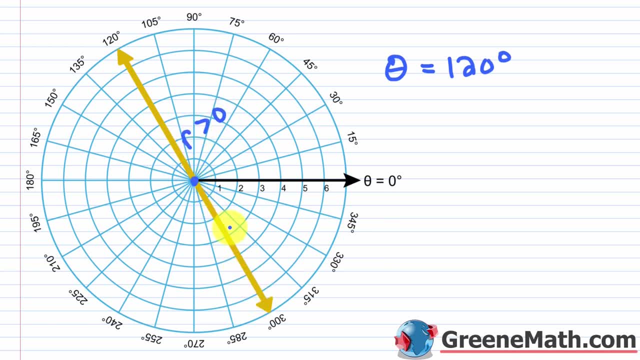 Okay, So essentially here r is greater than zero, And then down here your r values are less than zero. Okay, So again, this part is a little bit confusing. Again, if the r value was less than zero and you had 120 degree angle, you would find that angle, you would turn around and you would. 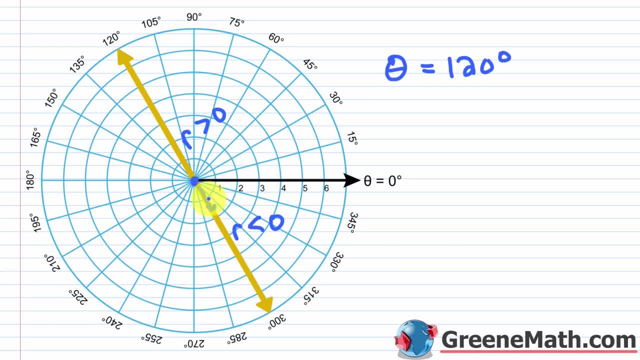 walk this way backwards. Now you could also draw the same line by saying that theta is equal to 300 degrees. Okay, So I know people would ask that, because if you have a negative r value, essentially if I gave you that one, well now the r value here would be positive. Okay, Because 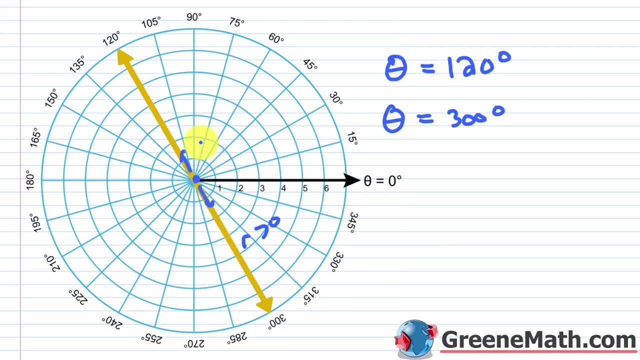 here I'll be walking forward, and then the r values going this way would be negative. Okay, So it's just a way to write the same line. Okay, But there's different conditions there, where r is going to be positive in one direction for this one and r is going to be positive in a different. 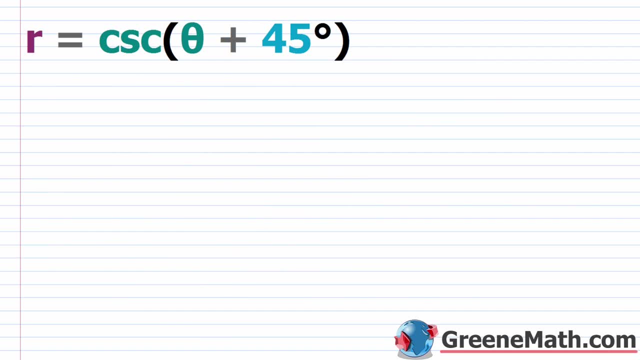 direction for this one. Okay, Let's look at a harder example. So this is one that takes a plus 45 degrees. All right, Whenever you see cosecant or cotangent or secant, go ahead and write it in terms of sine or cosine and see if that makes anything easier for you. Okay, Remember. 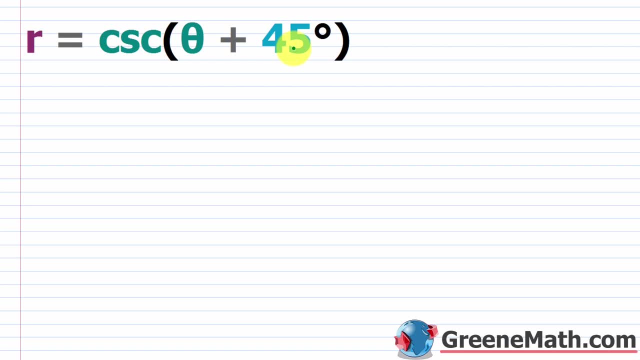 when we worked with our trigonometric identities. that was the general strategy. Okay, So that's what we're going to do here. I'm going to say: r is equal to. we know that one over the sine of theta is equal to the cosecant of theta. Okay, That's the relationship. So I'm going to say: this is one. 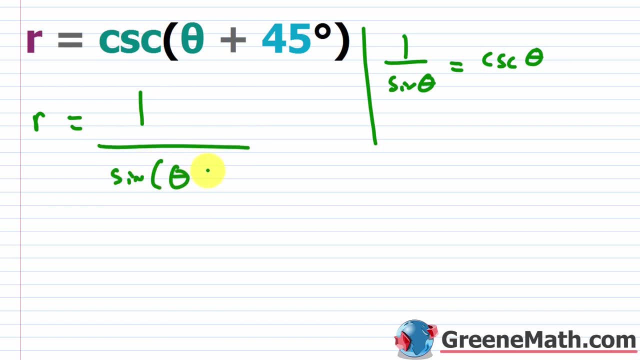 over the sine of theta. Okay, So that's the relationship. So I'm going to say this is one over the sine of theta plus 45 degrees. Okay, Now, from here I can multiply both sides by this sine of theta plus 45 degrees And that's going to give me that r times the sine of this theta. 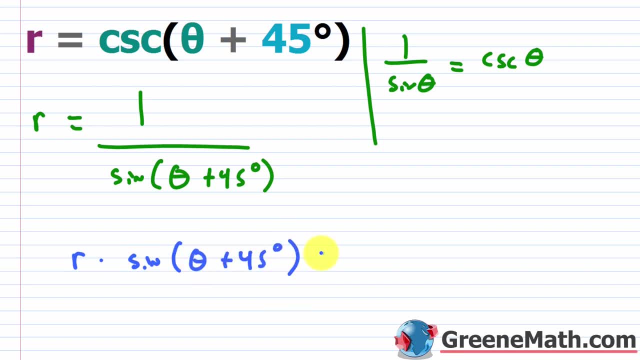 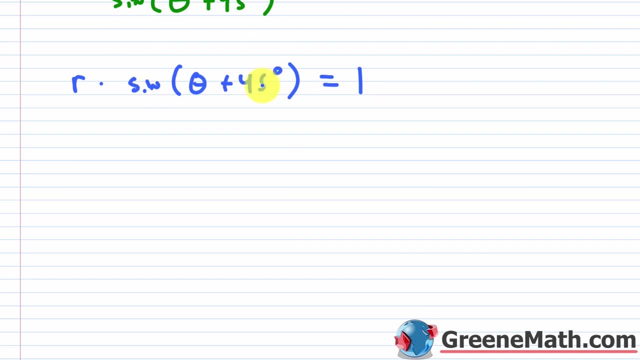 plus 45 degrees, Okay, Is equal to one. Now, again, again, again. we know that we can't just distribute this sine inside right. We know that we have a sine sum identity and we need to use that here. Okay, So to do that, I'm going to put some brackets around this guy and remember how. 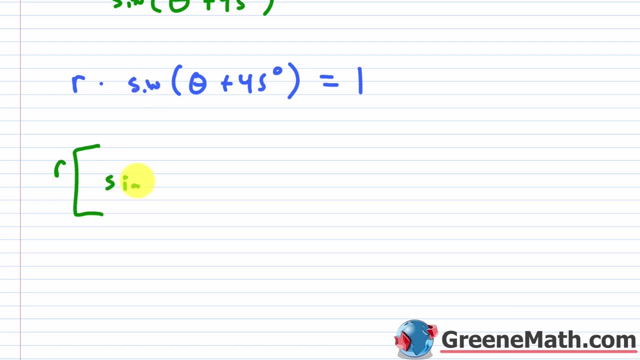 this identity works. It's the sine of the first guy, So the sine of theta times the cosine of the second guy, So the 45 degrees. then you're going to have, plus you're going to go- the cosine of the first guy, which is theta times the sine of the second guy, which is 45 degrees. Okay, So go ahead. 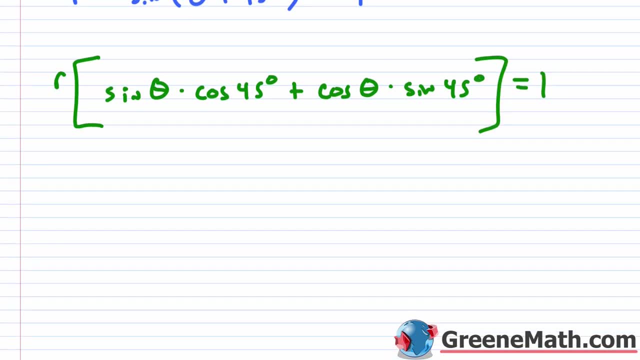 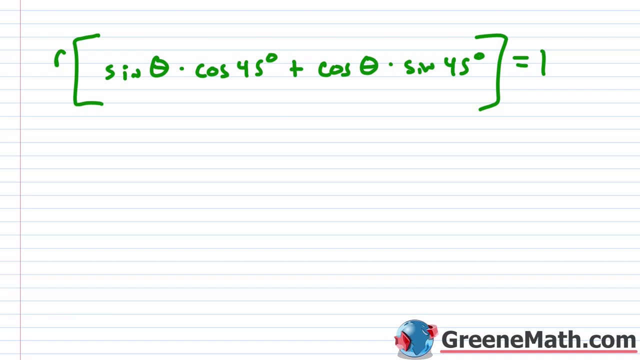 and close that down, This equals to one. Okay, So from here you see that it's getting a little bit easier, because we know that we're going to have a sine of theta plus 45 degrees. Okay, So from here, the sine of 45 degrees and the cosine of 45 degrees is squared at two over two. So all you. 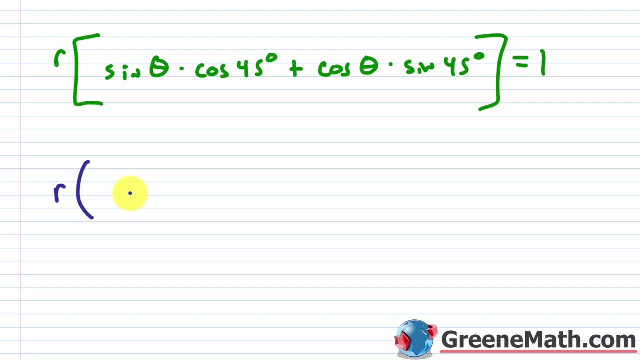 have to do is replace that. So I'll say r times- I'll just use some parentheses here. I'll say the square root of two over two and then times the sine of theta. Okay. Then plus, I'll say my square root of two over two times the cosine of theta. Okay, And this equals one. So from here, 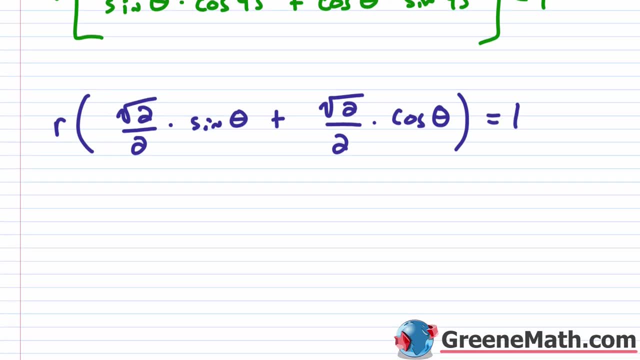 I need to do two things. Remember: we have this relationship where x is equal to r times cosine of theta and y is equal to r times the sine of theta. Okay, So if I distribute this r into each term, you notice that I could replace r times sine of theta with y and r times cosine of theta with. 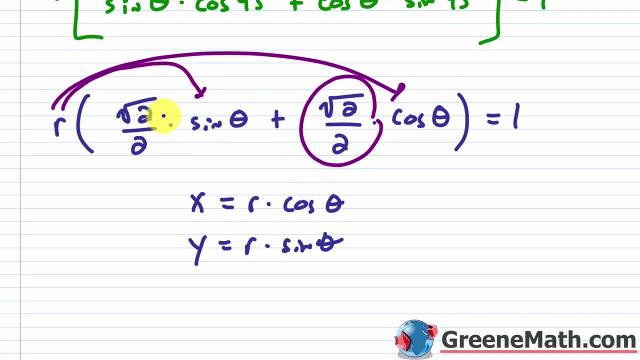 x. Okay. Also, I'd want to factor this guy out at the same time. I know I'm doing two steps in one, but I think you're strong enough to get that Okay. So what I'm going to end up doing is I'm 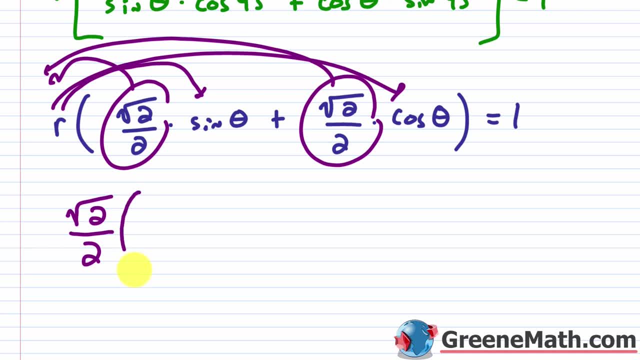 going to pull this out. So I'm going to say I have the square root of two over two, and then I'm going to distribute the r in, So I'm going to have r times the sine of theta, and then I'm going to 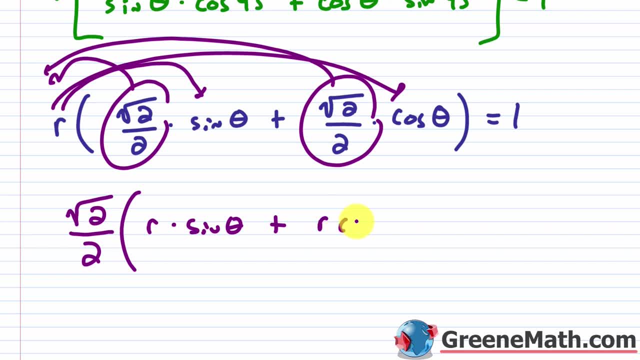 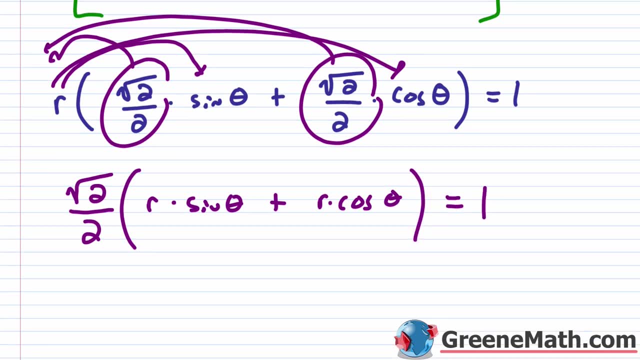 times sine of theta, and then plus, I'll have r times cosine of theta, And of course- let me make these parentheses a little bit better- I'll say: this is equal to one. Now, from here again: r times sine of theta, that's just y. r times cosine of theta, that's just x. So what I'm going to do is: 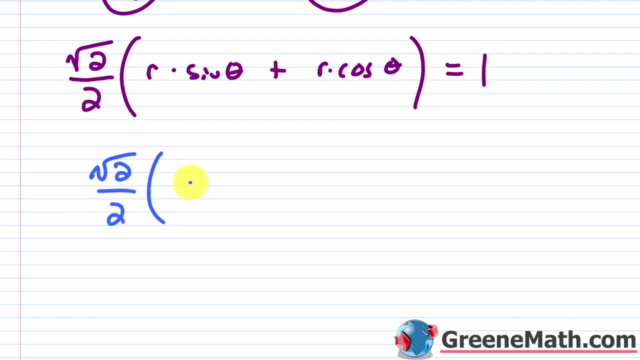 say, I have square root of two over two times, I'll have basically y plus x. You could rearrange that as x plus y- it's really up to you- And then I'll say: this equals one. Now, what I'm going to do is: 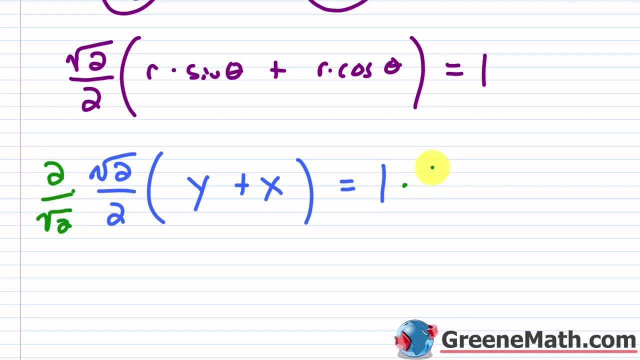 two over square root of two. So times two over square root of two, this is going to cancel And this is going to give me. I'll just go ahead and write this: as x plus y is equal to, I'll have two over square root of two. And of course, we always want to rationalize the denominator. Let 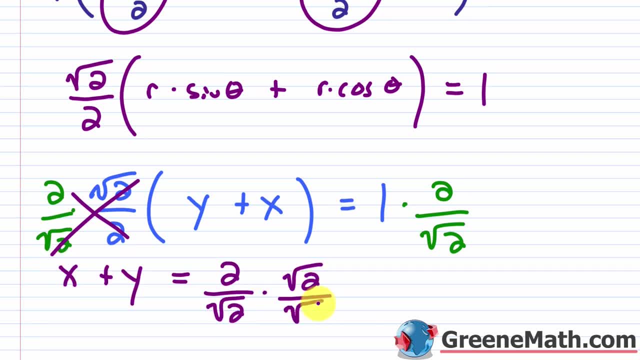 me move this over a little bit. So I'll multiply this by the square root of two over the square root of two, And what's going to happen is this: down here would become two, So this would be two, And up here this would be times the square root of two. Well, notice that now you can cancel. 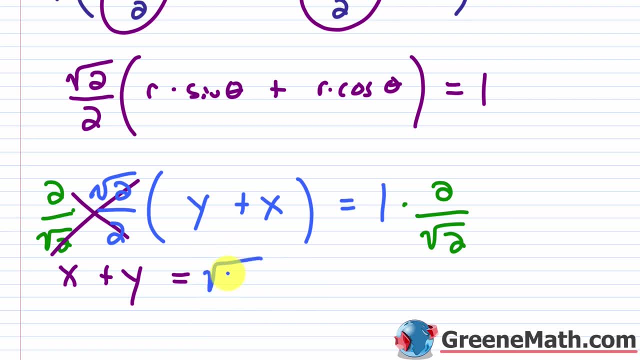 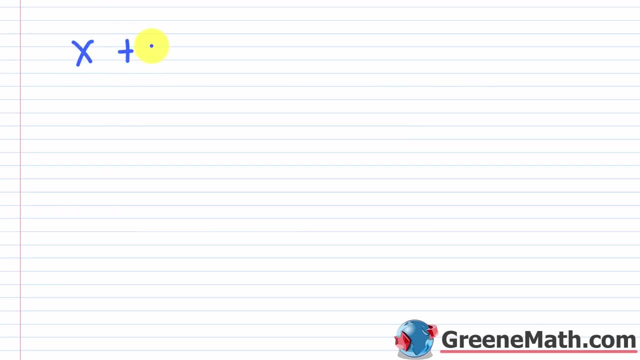 this with this. So I'm just left with the square root of two. okay, So here we have: x plus y equals the square root of two. Now let's talk about graphing this. So if we have x plus y is equal. 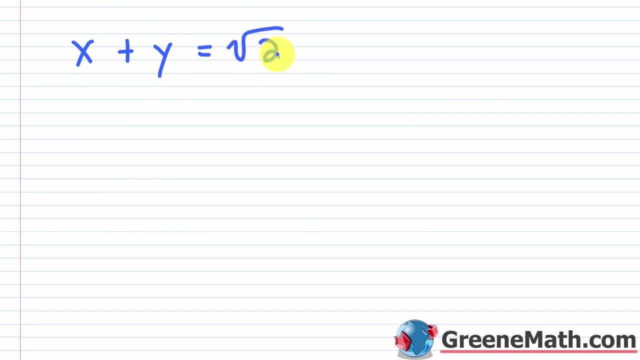 to the square root of two. from here I can figure out that my x-intercept would be what. Well, if I plugged in a zero for y, I would basically say that the x-intercept would be square root of two comma zero, And then basically my y-intercept. my y-intercept would be what? 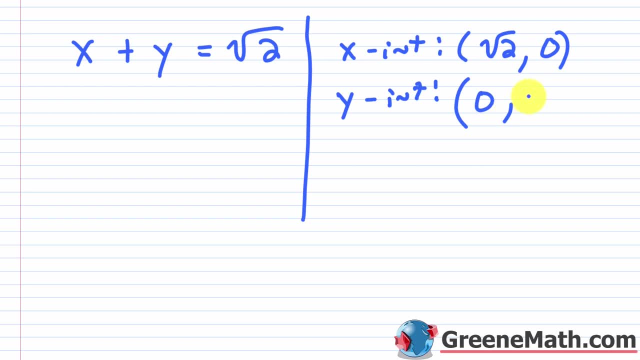 It would be zero, right? if I plugged that in for x comma. square root of two. okay, So again, these are easy to convert over. Now, the square root of two is something you have to approximate. Most people will say this is about 1.41, okay, So I'll go ahead and say that I have about 1.41. 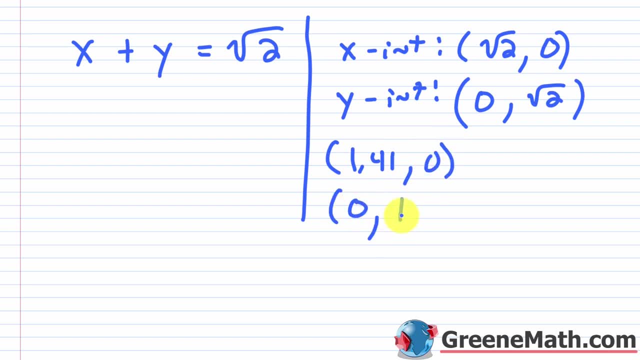 comma zero, and then I'll have zero comma about 1.41,. okay, Now let's say we wanted to convert these over to polar form For this one, I know that if I just plug in the square root of two, 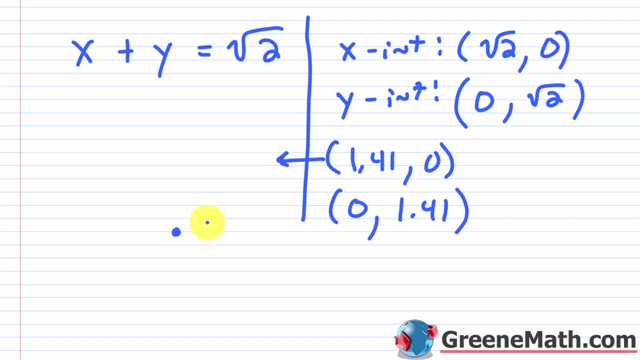 I just start at the origin and I'm just going to the right by 1.41 units. my angle is going to be zero degrees and my r-value is going to be 1.41.. So this is 1.41 comma, zero degrees. okay. 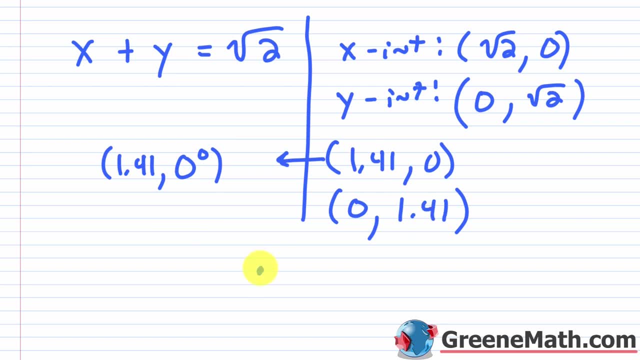 For this one I'm going to be going up, So from the origin I'm going to go up by 1.41 units, okay, So my r-value again is 1.41, and my theta value- here the angle, if I think about it- this: 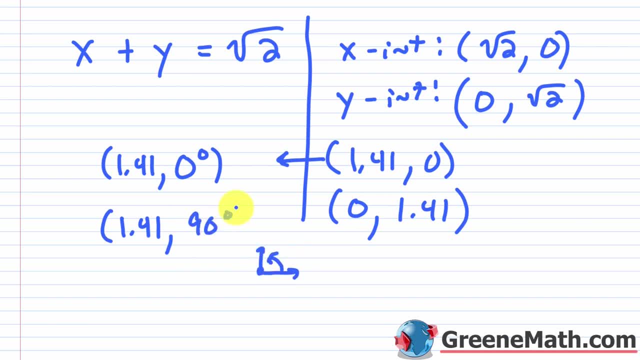 way right. that's going to be 90 degrees, So this is 1.41 comma zero degrees, So I'm going to go up 90 degrees. okay, Now you can go back and check this. Let me grab this real quick. We'll come back. 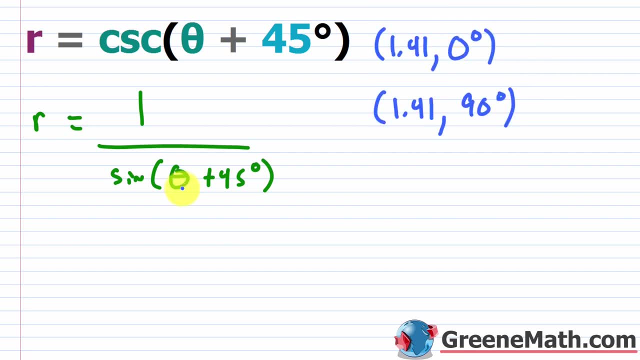 up here and paste this in. You can check these real quick. If you put in zero degrees there, the sine of 45 degrees is square root of two over two, okay, And if you think about it, you have one divided by that. so you're just flipping it and so you're going to end up with 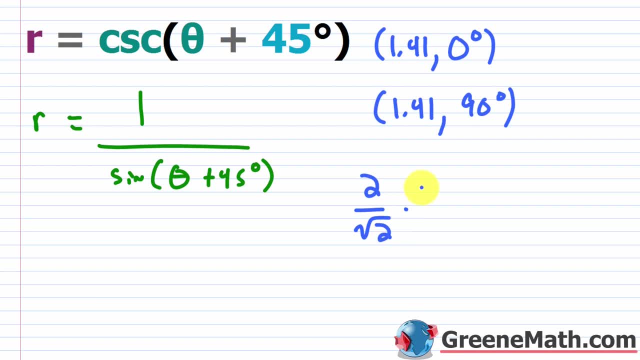 two. You're going to end up with two over the square root of two. Again, rationalize the denominator, okay, And you're going to end up with just the square root of two. okay. So a zero degree angle for theta gives me square root of two for r, okay, So we know that. Then the other. 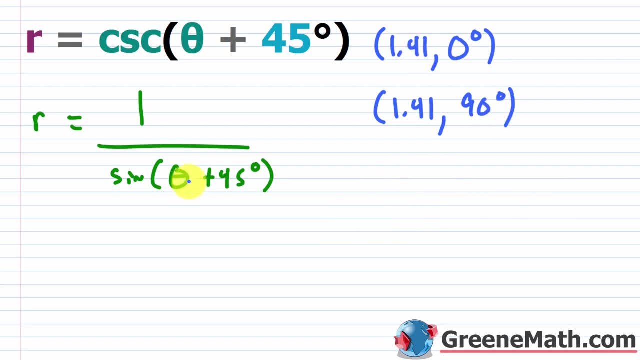 one. you can do this one. You plug in 90 degrees there. Well, 90 degrees plus 45 degrees gives you 135 degrees. You still have a 45 degree reference angle. so it's going to be the same thing, right. 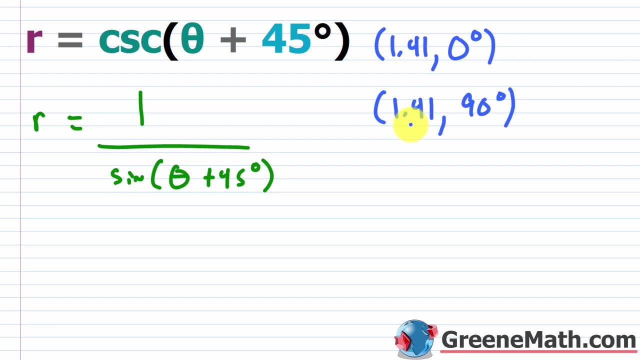 So basically, I'm going to end up with an r-value of square root of two. okay, Now, if you wanted one other point, you can think about your unit circle here. It's something that would work pretty nicely. You know that the sine of 30 degrees is equal to one half. 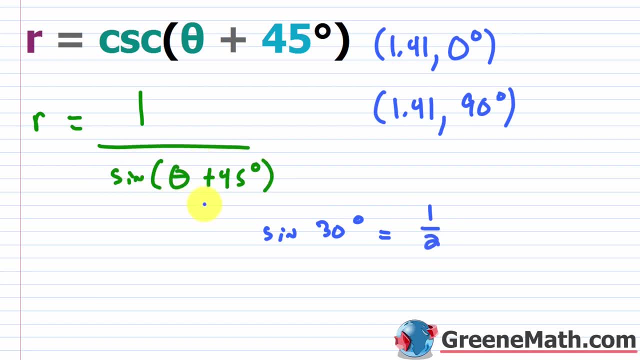 And so if I could make this bottom part one half, okay, somehow, someway, one divided by one half would be two, That would be a nice point to plot, okay. So what I could do, I could think about. okay, well, sine of 150 degrees. 150 degrees has a 30 degree reference angle. Sine of 150 degrees. 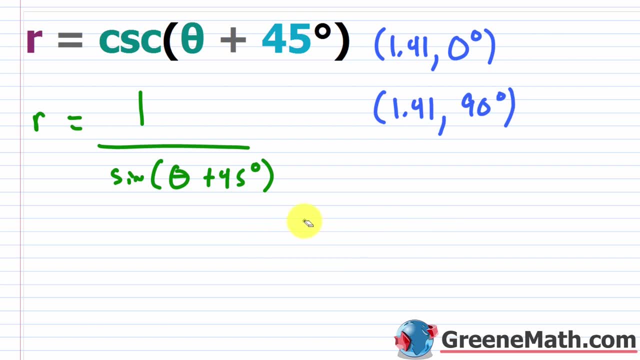 would also be a half, And what I could do is I could add 105 degrees, So I could put 105 degrees in there, okay, So I would have sine of 105 degrees plus 45 degrees is 150 degrees, okay. 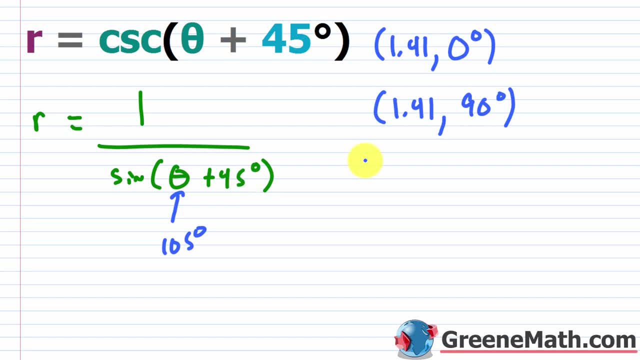 And the sine of 150 degrees is a half. So then your r-value there would basically be two, right, Because one divided by half is two And the theta value here don't plug in 150 degrees. It's what you're putting in here for theta. okay, So theta is 105 degrees, That's what you put in there, Be. 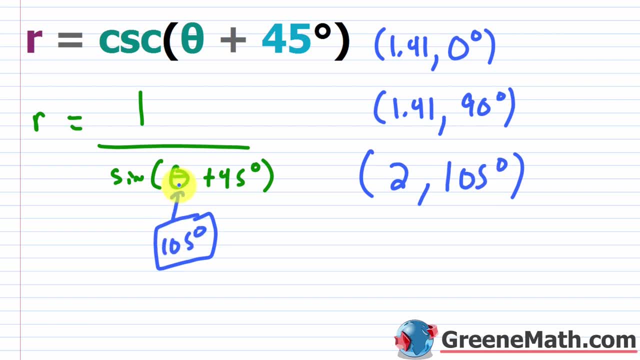 very careful. A lot of students make that mistake When you're plugging something in for theta. that's what's going in here. I am plugging in 105 degrees. I am not plugging in 150 degrees. 150 degrees is the result that comes from. 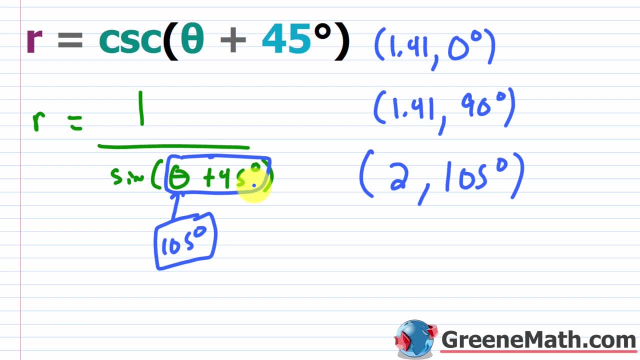 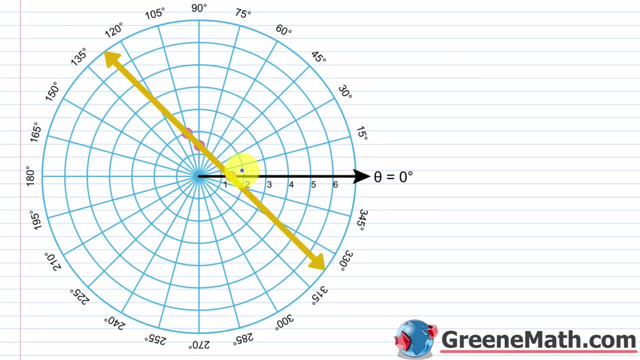 adding 45 degrees to 105 degrees. okay, So very important to make that clear. Now, once you have these three points, you can go ahead and sketch this guy. So let's go ahead and say that this point right here is going to be my point. 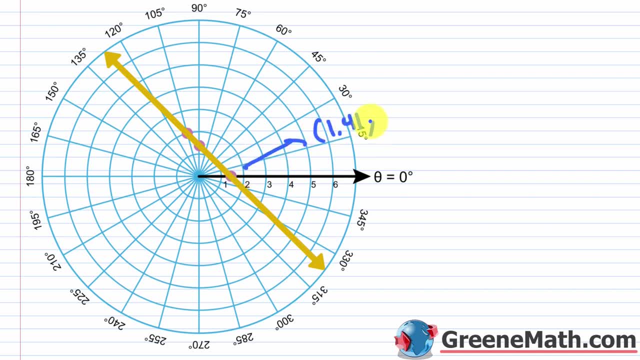 which is an r-value of, let's say, 1.41 approximately. And then I'll say: the theta value is zero degrees. okay, So that's one point. Then this point right here is going to be my r-value of 1.41, okay, So you notice how it would be on the same circle there. okay, And then basically, 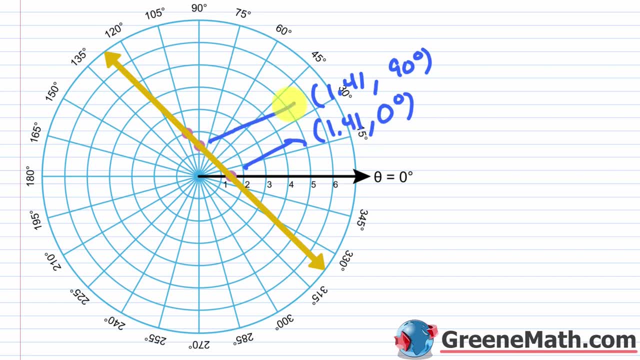 the angle here is 90 degrees, okay, So you can see that. So let me draw an arrow to that. And then also, we have this point right here: If you go out to a circle with a radius of two and we swing around to this 105-degree angle- remember, you want a 105-degree angle. 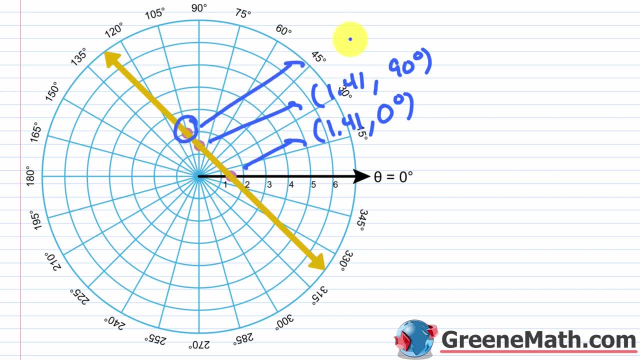 not a 150-degree angle, but a 105-degree angle. this guy right here would be a 0.2. So you would have 2,105 degrees. okay, You're just finding some points and then sketching a line through the points. All right, let's also talk about horizontal and vertical lines. to wrap, 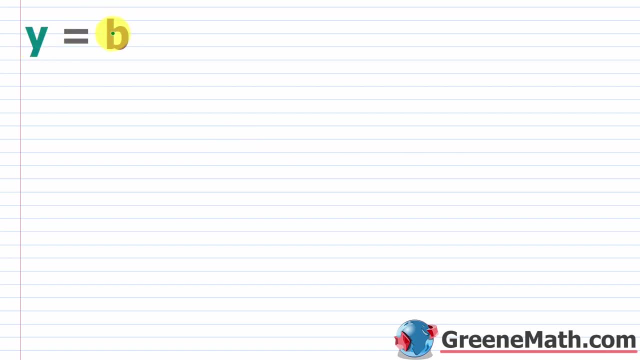 things up. So if you get something like y equals b, you know this is a horizontal line, right? So basically, no matter what the x value is, y always equals that constant b. okay, And essentially for this I would just say: okay, well, I have r times sine of theta, just plugging that in. for y there is. 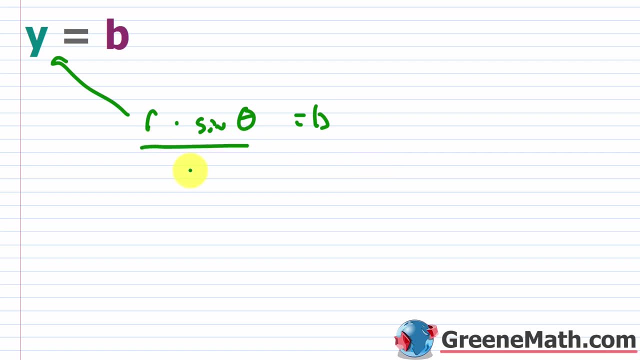 equal to b And I would divide both sides by the sine of theta. okay, So both sides by the sine of theta. And so if you see something like r is equal to some constant b over the sine of theta, you know that you have a horizontal line. 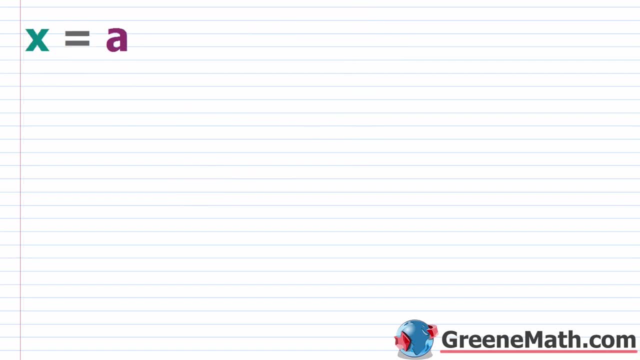 Okay, that's very clear, And I'll show you an example of this in a moment. Let's also look at the vertical line. So you know, if you have something like x equals a, this is a vertical line. no matter what the value is for y, x always equals that constant a. So here I'm just going to 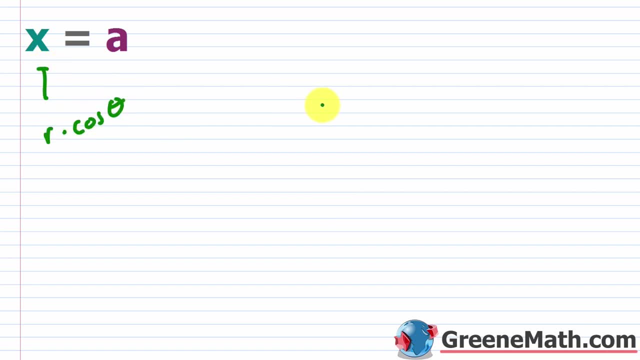 plug in r times cosine of theta And essentially I would have r times cosine of theta is equal to a. divide both sides by the cosine of theta, So divide by the cosine of theta, So you get r is equal to a over the cosine of theta. okay, So this is your vertical line. 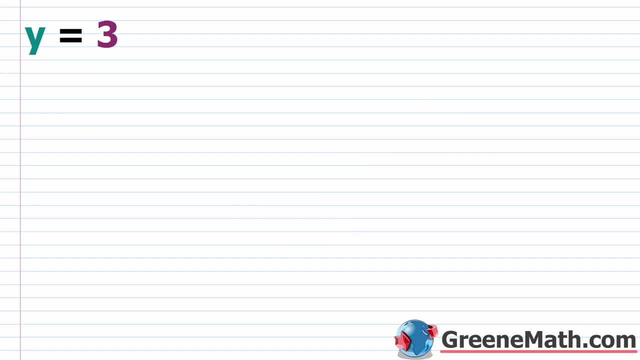 All right, let's look at two quick examples. So we see here we have y equals three. To convert this over again, if it's a horizontal line, then I know it's going to be. r is equal to. you're going to. 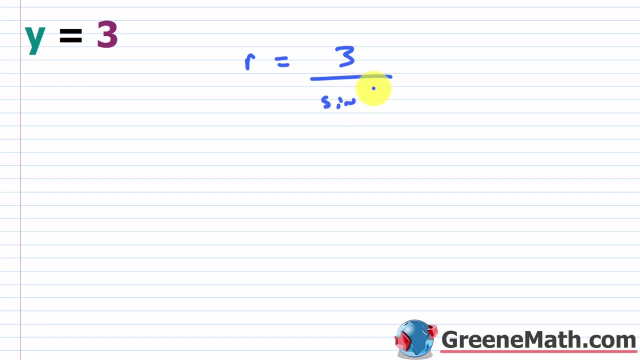 have this constant here, which is three over the sine of theta. Okay, that's all it is. And to graph this, it's no different than when you graphed it on the rectangular coordinate plane. you would basically just go up from the origin- three units, okay, by this number of units and make a horizontal. 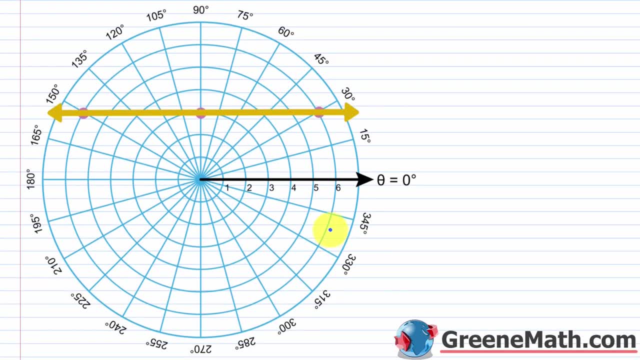 line. If you go here and you look at this guy, you're going to see that the horizontal line is. You can start here. I go up to a circle with a radius of three. so I'm right there. So, basically, one point of the line- and we'll verify this in a second- would be three for the radius. 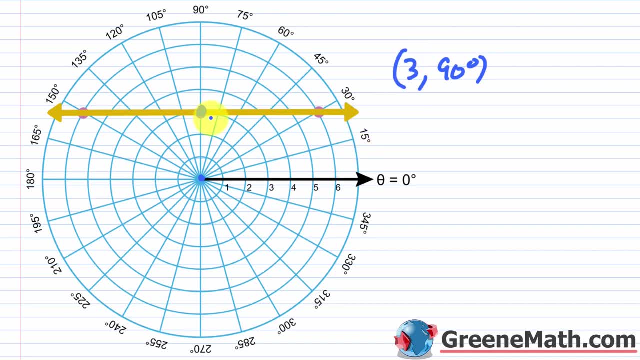 and then 90 degrees for the angle, okay. So that guy would be on that line And then essentially you would just draw a horizontal line there. Some other points: you would have six comma. you would have 30 degrees, okay. And then another point: you could see that you would have six. 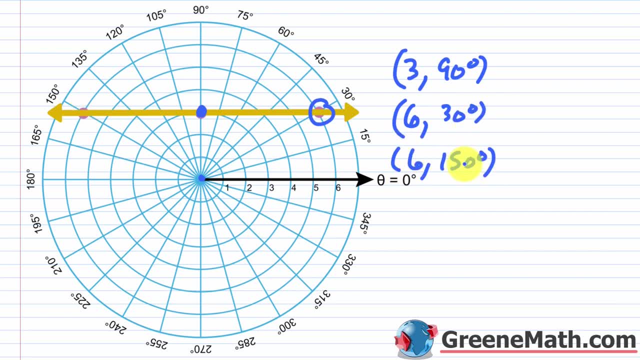 comma 150 degrees. Notice that 150 degrees has the same reference angle. And also, since sine is positive in quadrants one and two, you would have six comma 150 degrees. And then- another point: it would have the same sine value, right In each case it's a half. So if we go back, 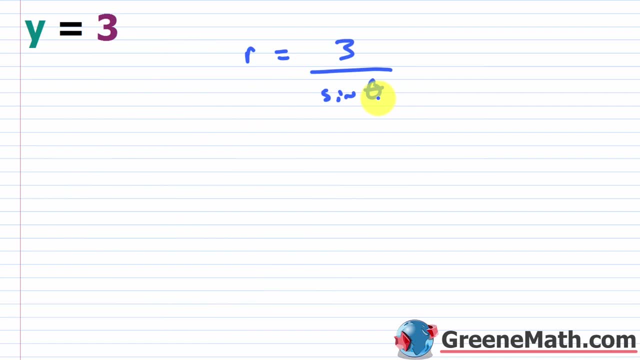 and we think about: does this work? Well, the sine of 90 degrees is one, So three over one is three, So that works right. Basically, if I plugged in 90 degrees there, my R value would be three. 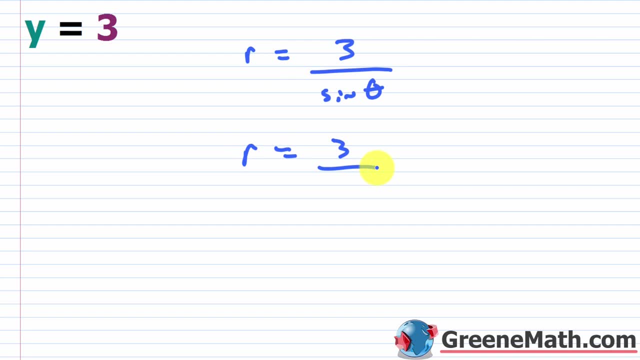 And then, if I did, R is equal to three over the sine of 30 degrees or the sine of 150 degrees. well, in each case this would be a half, And essentially you would have three times two, which is six, okay, So there you would get six comma 30 degrees. 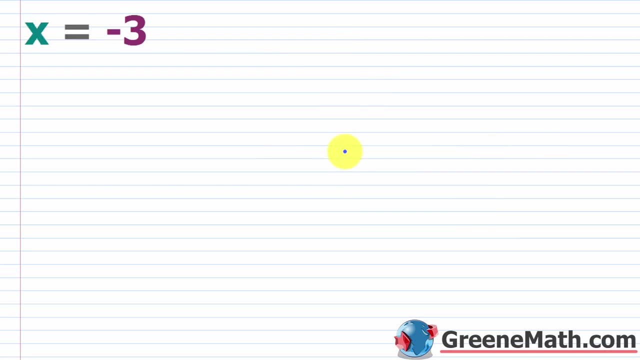 or six comma 150 degrees, All right. so lastly we have: X is equal to negative three. So, following the formula, we'll say R is equal to, we'll say, negative three. We'll go ahead and say that's divided by the cosine of theta. okay, So before we go to the graph again, if you think, 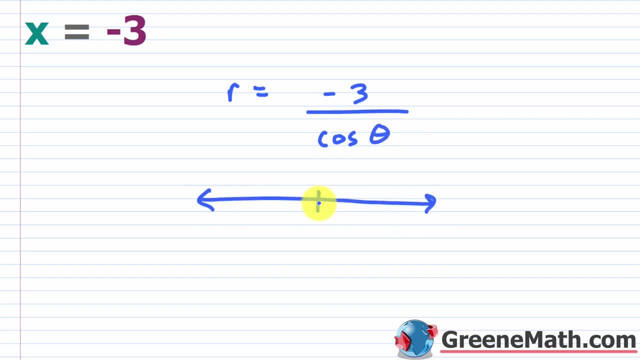 about a point that's going to work. think about your coordinate plane. If this is zero, comma zero. if I want the X intercept which is going to occur at negative one, negative two, negative three. So this point right here on the rectangular would be negative three. 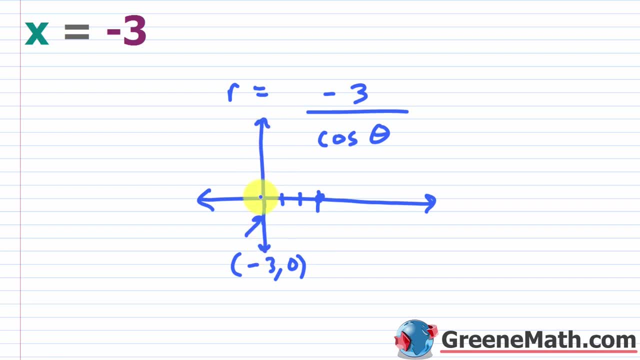 comma zero, right? So if I'm drawing a vertical line, this is where it's going to cross. Now, if you think about this, this is going to be what It's going to be: an R value of three, And then again this angle here is going to be 180 degrees. So you can stop and plug that in and 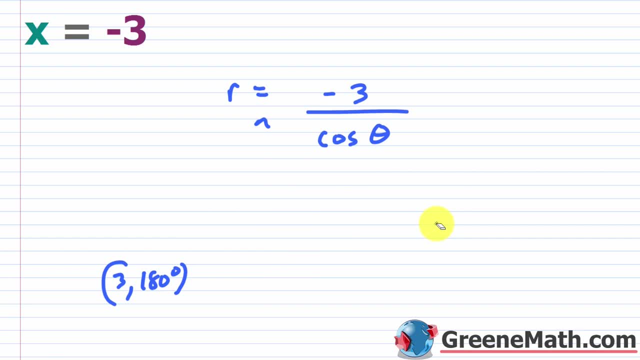 see if it works. The cosine of 180 degrees is negative one, right? So essentially we would have negative three over negative one, which is going to be equal to three. okay, So that gives me that point right there. You could grab other points, You know. 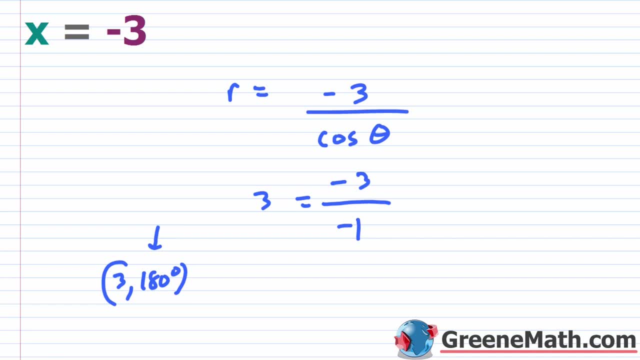 that the cosine of 120 degrees is negative a half And then also the cosine of 240 degrees is negative a half. So if you did something like, let's say, 120 degrees and then also 240 degrees, what's going to happen is you're going to be dividing by negative one half. 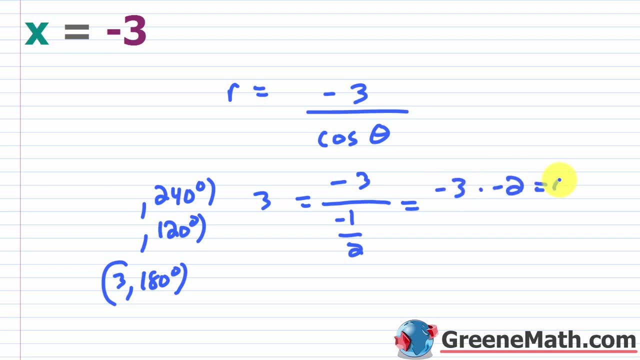 which is like negative three times. you'll do negative two, which is six. Okay, So this would be some points, And I know that six and three don't match up, but remember, we're on the polar grid, So if we look at this guy, you can see that from here. 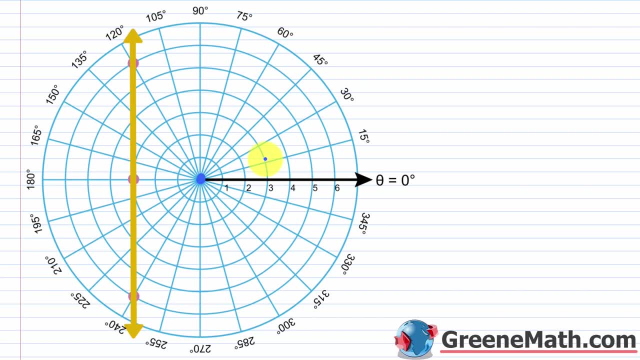 You're basically going to go out to a circle with a radius of 3 and then swing around to 180 degree angle. So there's your x-intercept as it would be on your rectangular coordinate plane. here It's going to be at 3 comma 180 degrees. Okay, from there You can basically make a vertical line. 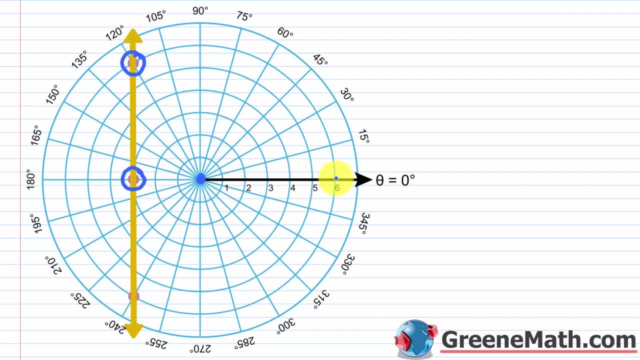 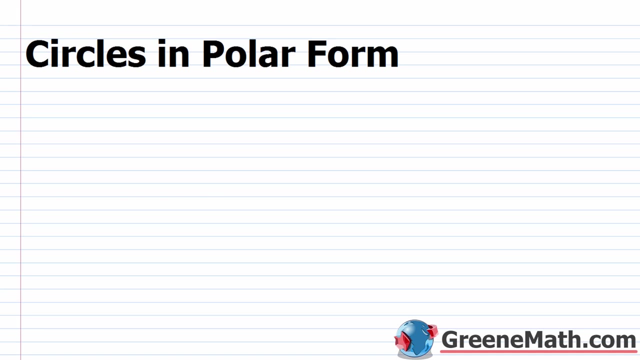 But I just want to show you again at this point right here Would basically be going out to a circle with a radius of 6, Swinging around to 120 degree angle. or going out to a radius of 6 and swinging all the way around Until you get to 240 degrees. So that's that point. there in this lesson We want to talk about circles in polar form. 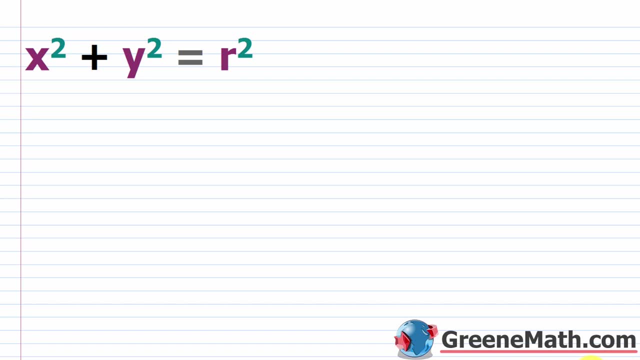 All right. So in this lesson we're going to learn how to convert back and forth between the rectangular form of a circle And the polar form of a circle. We'll also look at some strategies to graph a circle on the polar grid. So i'm going to start off with a circle whose center is at the origin. 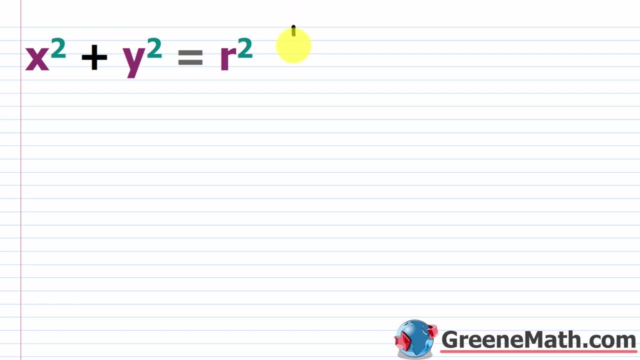 This is the easiest scenario and we're going to think about converting this back and forth now. first and foremost, When you work with polar form, you have that all okay. So remember, if you have something like the cosine of theta, We say this is x over r. if we have the sine of theta, 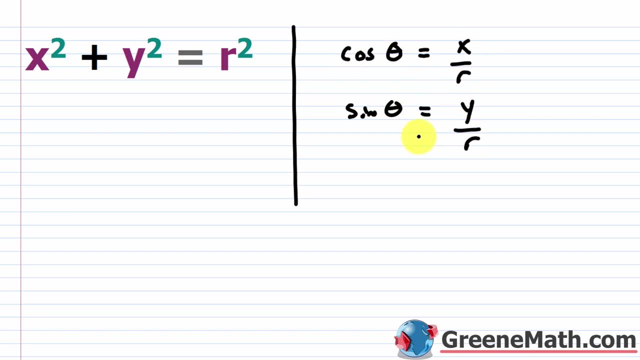 We say this is y over r, and if you multiply both sides by r in each case, You would get r times cosine of theta is equal to x, and then you would get r times sine of theta is equal to y. Okay, so what i'm going to do here, instead of having this r squared in rectangular form, 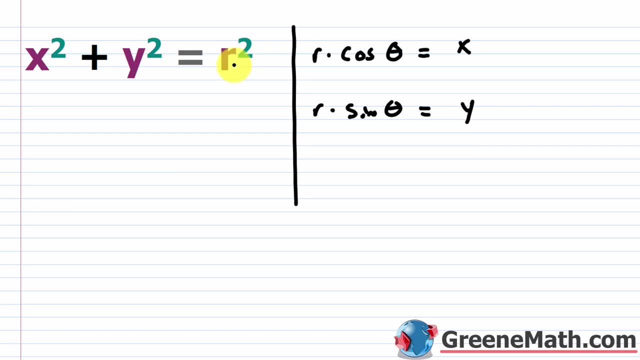 I'm going to replace this with an a. okay, So the a is now going to be the radius of a circle. Okay, so i'm going to say this: is x squared plus y squared is equal to a squared. So that's typically the letter chosen in your textbook. 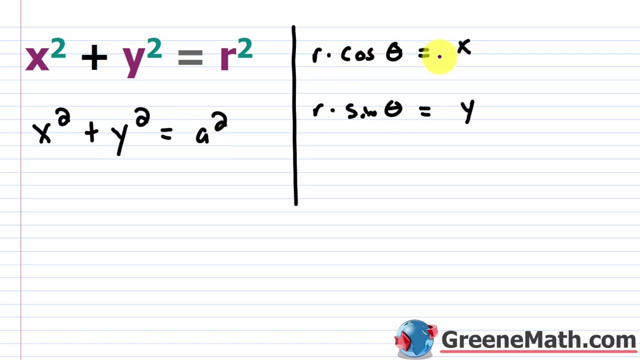 So what i'm going to do now is think about the fact that, okay, if I want to convert this to polar form, I can always plug in r times cosine of theta Anywhere I see an x, and I can plug in r times sine of theta anywhere I see a y. 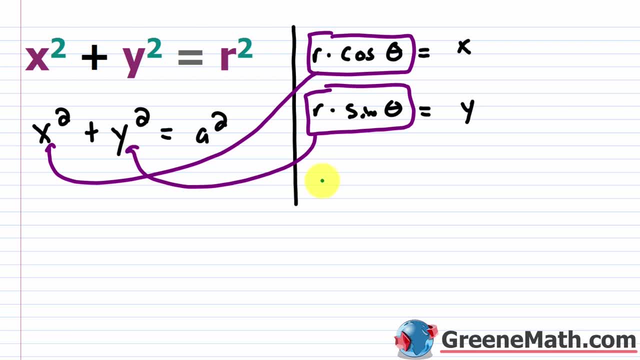 Okay, so this is the longer way. some of you already know that x squared plus y squared is equal to r squared. Okay, so this is the longer way. some of you already know that x squared plus y squared is equal to r squared. Okay, we use this when we convert our rectangular points to polar points. 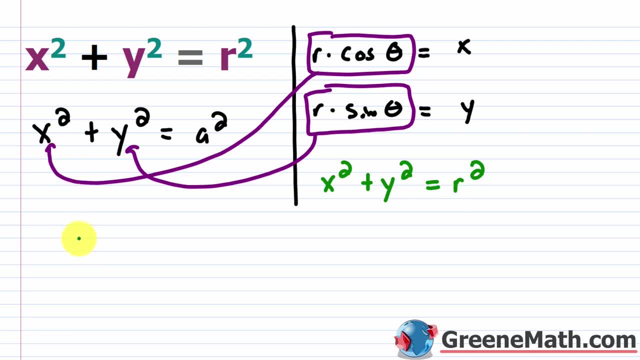 So we already know this relationship, but let me show you this real quick. So if I plug in here, I would have r times cosine of theta being squared, Then plus you would have r times sine of theta being squared Equals a squared. Okay, so because this is multiplication here you can bring this in. 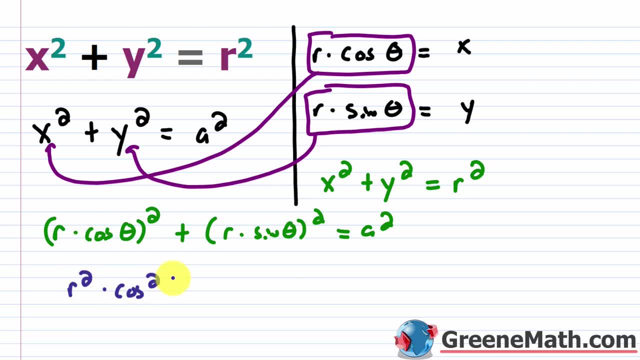 So you can say this is r squared times cosine squared theta. Then plus r squared times sine squared theta, And this is going to be x squared times sine squared theta And this is going to be equal to a squared. Now the idea here, if you want to show that basically this side here is basically r squared. 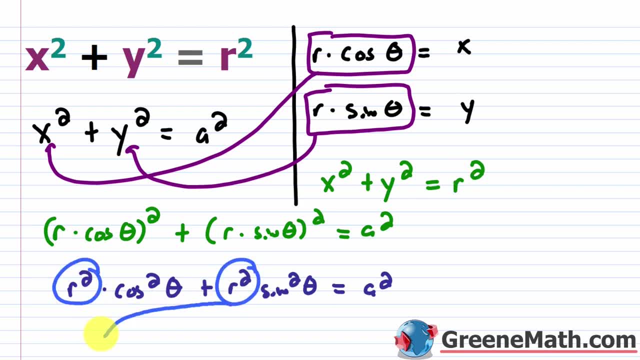 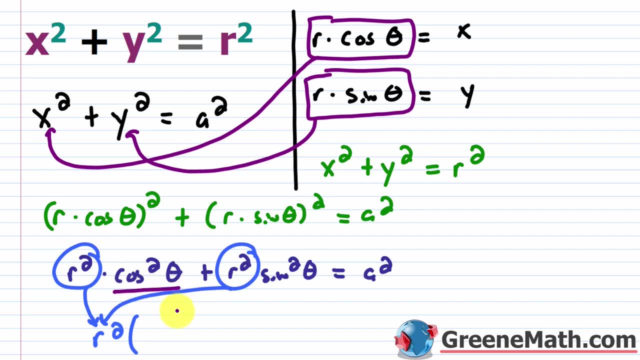 Then you can just factor this out. Okay, so pull this out in front of a set of parentheses. So r squared here times the quantity what's left. Well, what I'm going to have is my cosine squared theta. So cosine squared theta. then, plus my sine squared theta, my sine squared theta, this equals a squared. 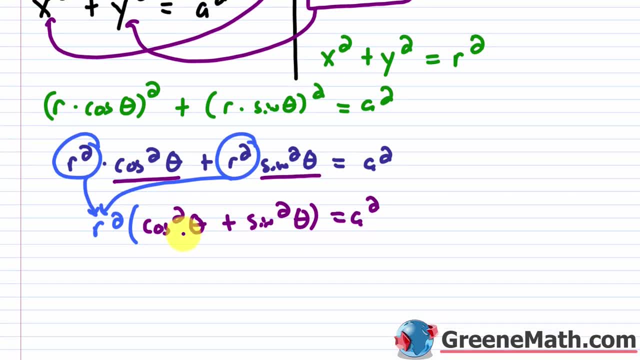 So let me scroll down for a moment, get some room going, And I want you to think about The fact that this is the pythagorean identity, where you have sine squared theta plus cosine squared theta is one right, And if you reverse that, it's the same. 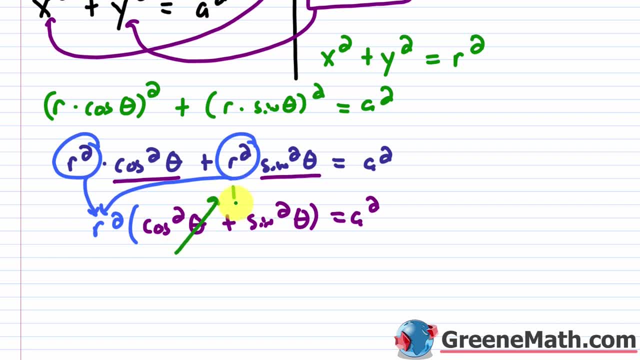 So this is one. so I can go ahead and just cross this out and say it's one, And you see that x squared plus y squared is just going to give us r squared. Okay, so now I have r squared equals a squared. Okay, and here comes the confusing part. 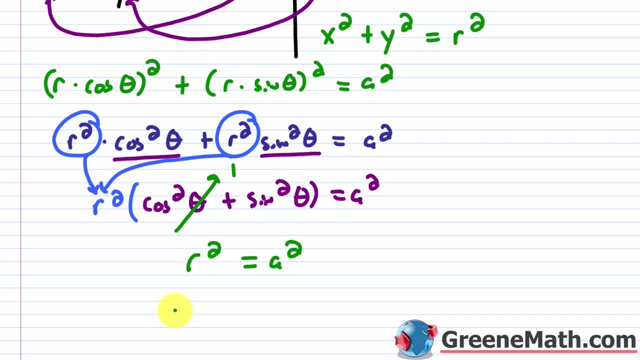 If I solve this for r, what I end up with is: I end up with: r is equal to plus or minus a. Now, this result here is confusing because when we work with this in the rectangular Coordinate plane, we don't have a negative radius. It doesn't make any sense. 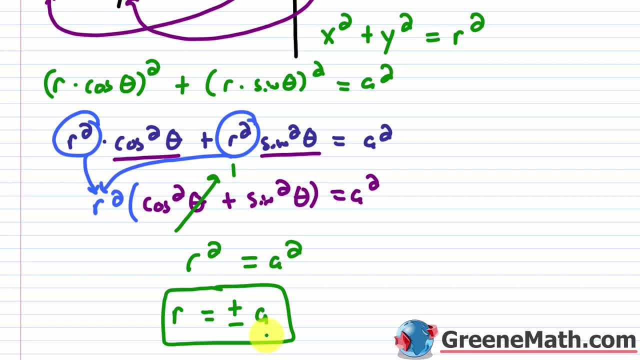 But if we think about this, in polar we can have a negative rate, so it's allowed. So basically, we're gonna see this. some books will actually write just r equals a, and I'll explain this when we get to a problem, How you're gonna end up with the same graph either way. 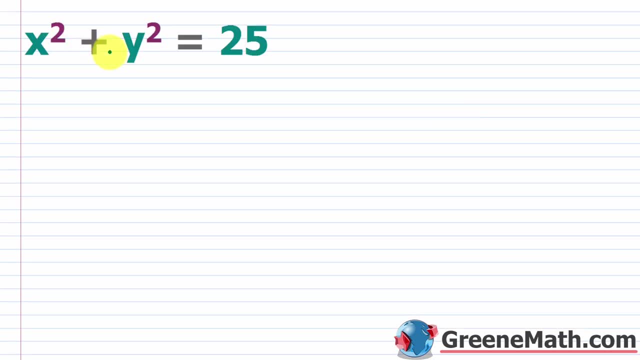 All right, let's go ahead and look at a simple example. So we have x squared plus y squared equals 25, So again this matches your format of x squared plus y squared is equal to, again, the radius. here We're gonna call it a, so a. 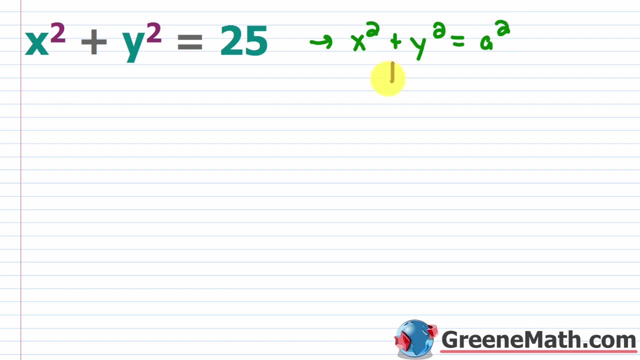 being squared. Okay, and this converts over to. you would basically have: your r is equal to plus or minus a, which you have to consider. Here's 25 is not a, it's a squared right. So what I would want to say is to convert this over. I could quickly just say this is: r is equal to. 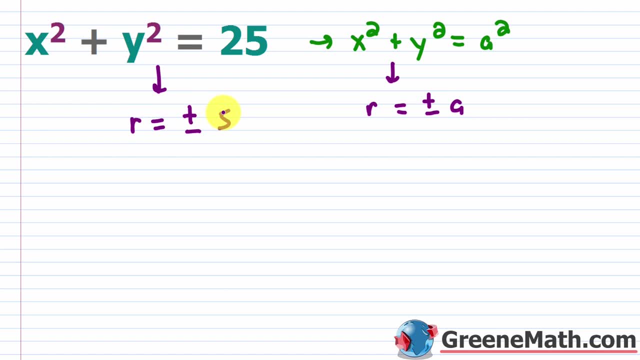 Plus or minus 5, right, That's all you would really need to do again. If you want to do this the long way, I want you to consider the fact that we just showed that R squared is equal to x squared plus y squared. Okay, so basically, I can. 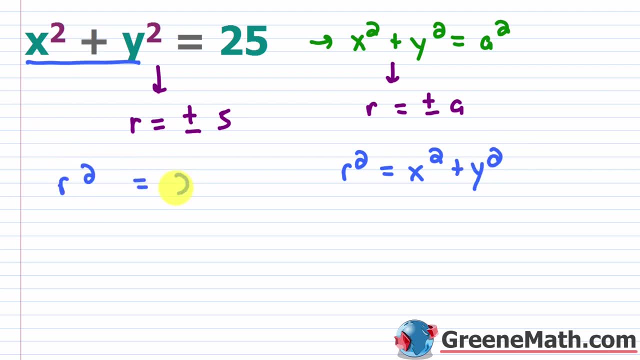 Replace that with my r squared, this equals 25, and if you solve for r, r equals plus or minus 5. So, however you want to do this, you can do it this way, Which is a bit longer, where you can just use your formula if you have it memorized. 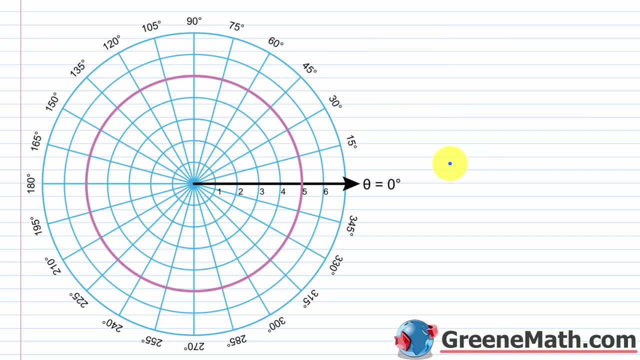 All right, let's talk about graphing this guy now. So essentially, people get a little bit confused. if you have something like r is equal to, let's just say, 5 for right now, What would I do? Well, there's no theta involved, people always trying to plot points with theta and R. 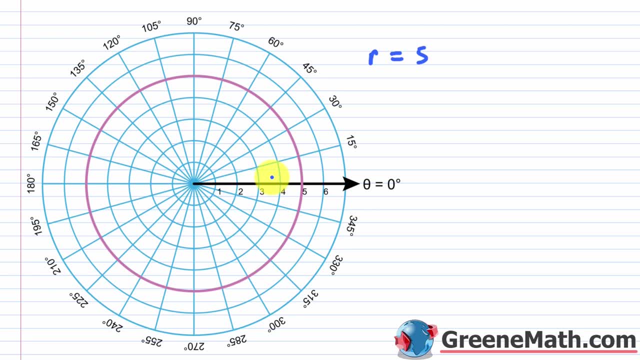 There is no theta. so that just means, no matter what the theta is, no matter what The angle is, the R value is always 5. so, starting from the pole- Okay, let's say that theta was 15 degrees- I just walk forward by 5 units, right? So I'm going to be on this circle with a radius of 5. 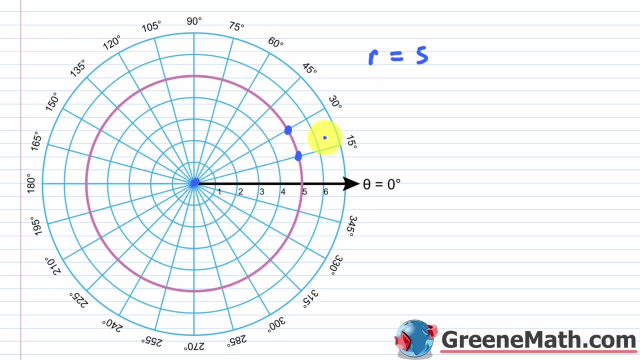 Okay, then if I was at 30 degrees, I'd be on a circle with a radius of 5, you know, so on and so forth. You're gonna end up basically tracing a circle through those points that are formed to get this graph here. 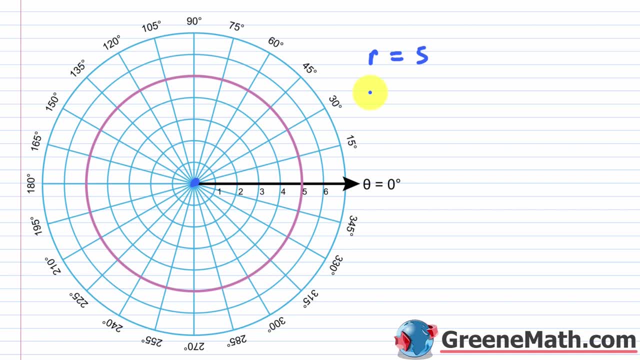 Okay, that's all you're doing. Now, if you consider, r equals negative 5, Remember if you had a point? Let's just say it was 5 comma 45 degrees. Okay, so that's going to be coming out to 5, a circle with that radius swinging to 45 degrees. That's right there. 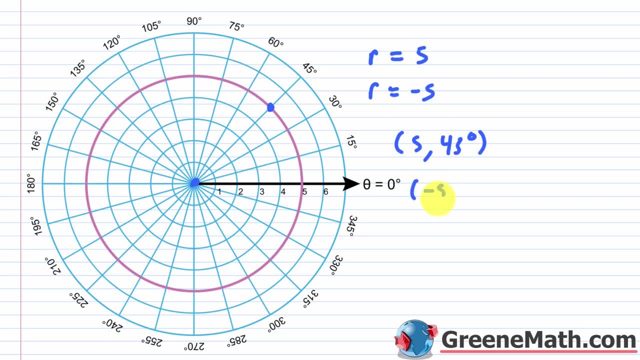 Okay, consider that you could locate the same point by saying you had negative 5 comma, 225 degrees, right? So, in other words, if I'm facing this way, right, I swung all the way around to this angle, right here. Okay, Well, what I want to do is go backwards now. 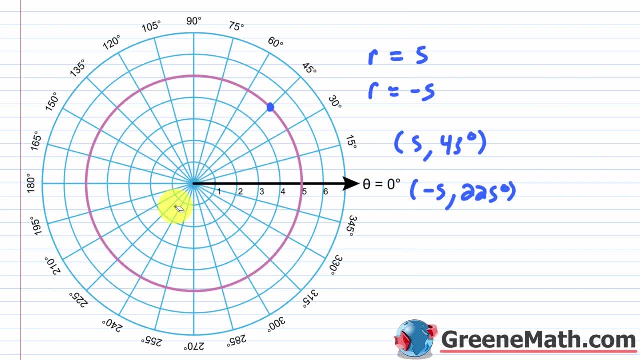 So I want to go this way by 5 units, So you can trace out the exact same points using that logic. So r equals negative 5. there would be the same circle, Okay. so that's why a lot of people will just drop this one and say okay. 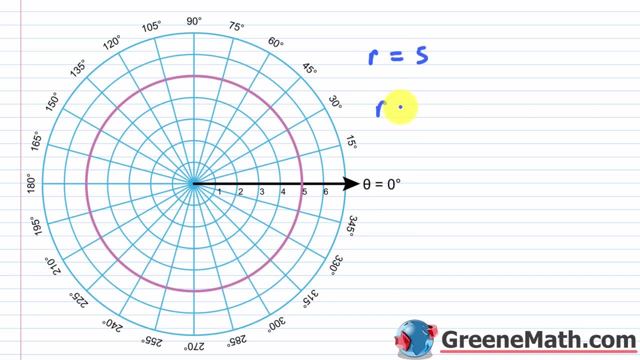 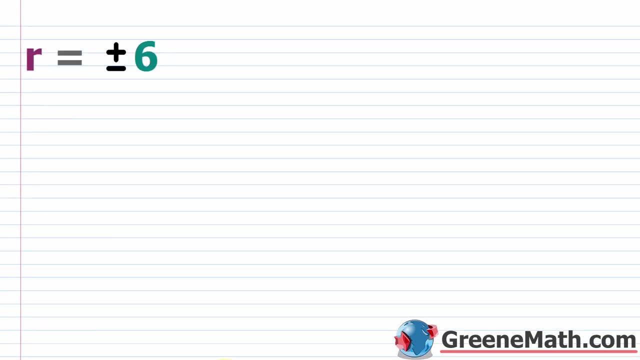 this is the graph of r equals 5, but again, some teachers want you to put r equals plus or minus 5, like this, just Because you can't have a negative radius with the polar grid. All right, Let's go ahead and take a look at an example where we have an equation of a circle that is centered at the origin. 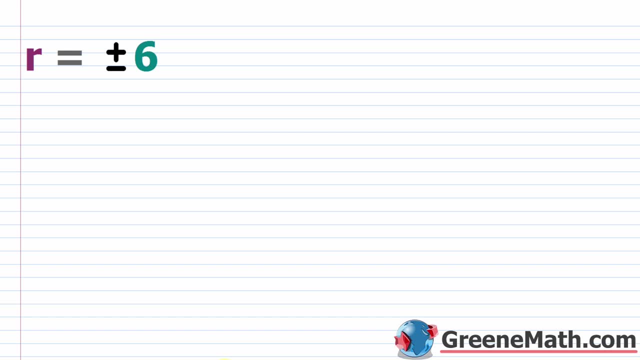 And it's given to us in polar form. we're going to put this in rectangular form. we're also going to graph this on the polar grid. so we have that r is equal to plus or minus six. and remember we can say that x squared plus y. 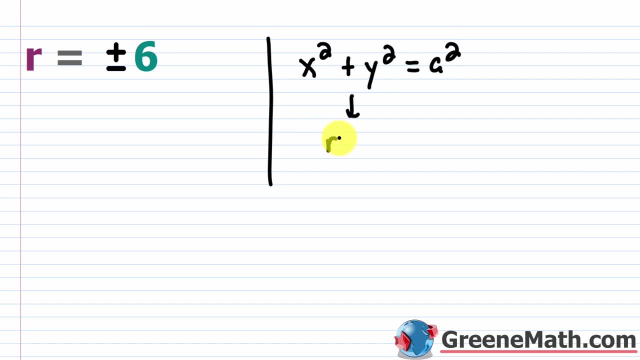 squared equals a squared can be converted to r equals plus or minus a. so now we're going backwards here, so we have the r equals plus or minus a. in this case a is six. we want to go to this form. so i would just say: i have x squared plus y, squared is equal. to go ahead and square a, a is six, that's. 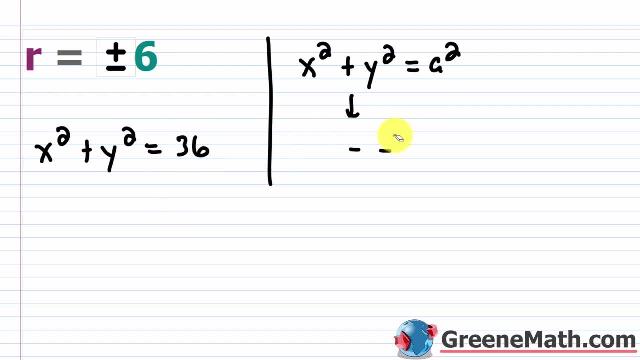 going to be 36. okay, another way you could do this. if you don't like using these formulas, or maybe they're too tough to memorize, you can just square both sides. that would give me that r squared is equal to: if i have positive six or negative six, and i square it, i get 36, remember, whenever. 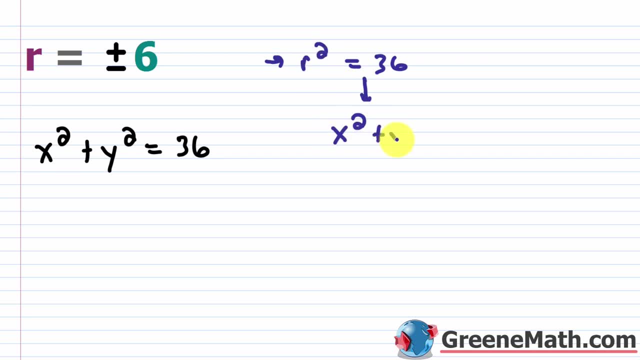 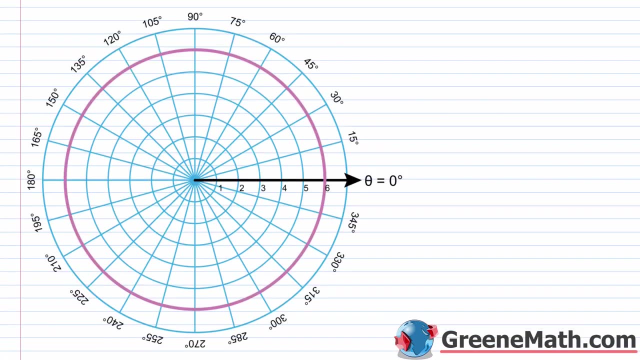 you have r squared. you can replace that with x squared plus y squared. okay, going over to rectangular, and this just equals 36. so either way, you're going to get the same answer. now, graphically again, this is very easy to do. so r equals plus or minus six from the origin or from the pole, if you want to think about it that way. 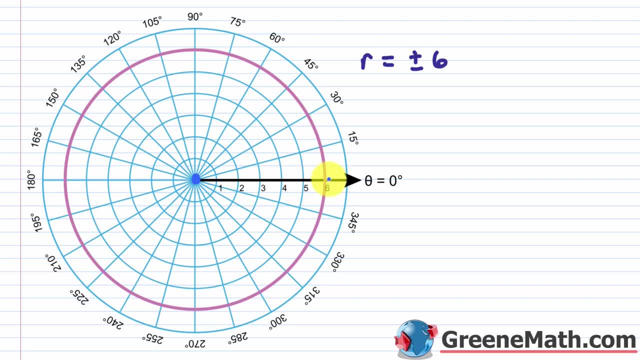 essentially, i'm just walking forward by six units. okay, so i'm going to a circle with a radius of six in each case, no matter what the angle is. okay, so i would trace out a series of points. okay, and again you can trace out the same points using a negative six for the radius. so then you sketch your graph. 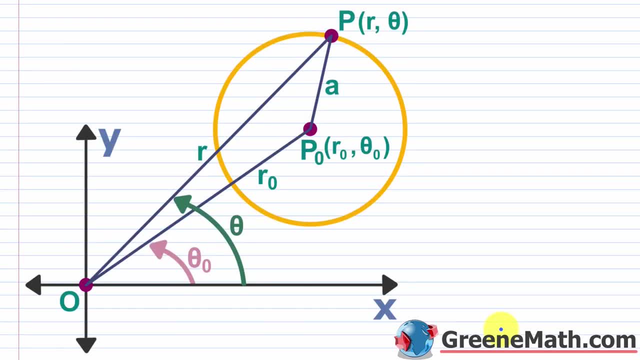 by tracing a circle and you're going to get the same answer. okay, so i'm going to go ahead and circle through those points and you're done all right. in most cases, we're not going to see a circle whose center is at the origin. a lot of times, though, the circle will pass through the origin. 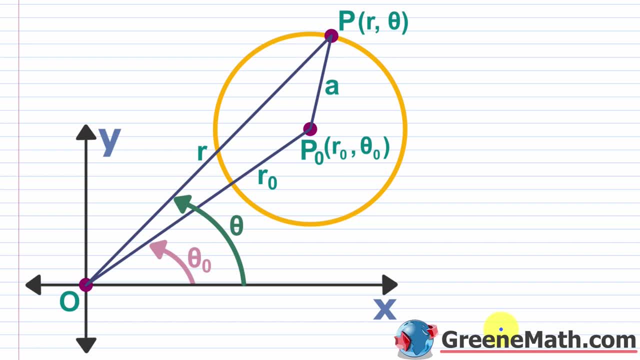 and so most of our problems will involve that scenario. so i'm going to start off with something generic here. you'll see this in most textbooks. let's say we had a circle that was not centered at the origin. okay, and essentially what i'm going to say is that the center of that circle 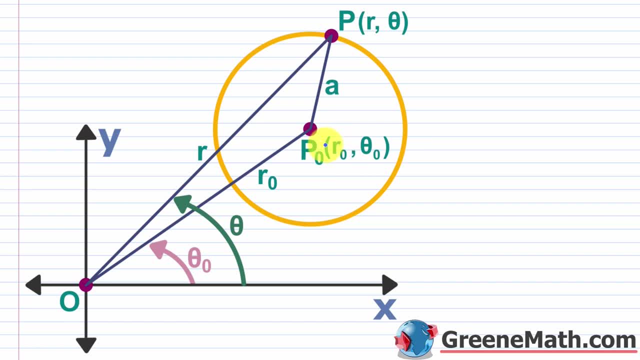 is going to be labeled as p sub zero, and then the polar coordinates for that point would be r sub zero and then theta sub zero. so the distance from the origin, which we labeled as o, to this point, which is the center, p sub zero, okay, would be r sub zero. so that's the length of this side, right here. 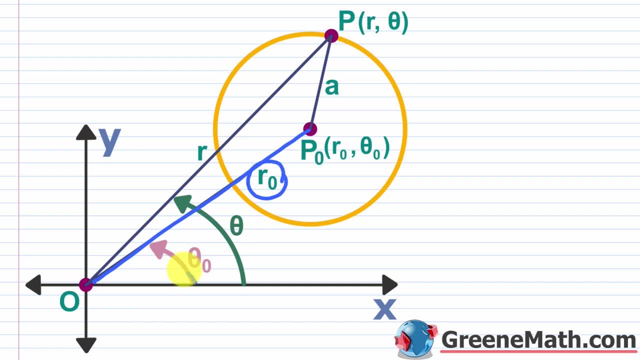 okay, so that's given by this r sub zero, and the angle here is going to be theta sub zero, okay, so we've got that part now. the other thing is we can have ourselves a little point on the circle, so let's call that p, okay, and the coordinates there in polar are going to be r comma, theta. 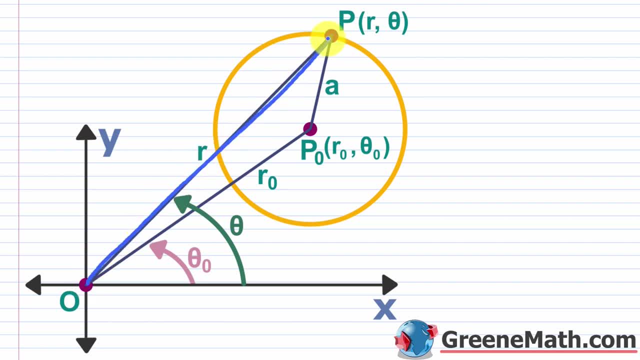 so the distance from the origin to that point is going to be r, comma theta. so the distance from the origin to that point, p okay- would be r. now the angle there, this guy right here- would be theta. so we have those two things. now, if i want to figure out what is the length of a, which is the 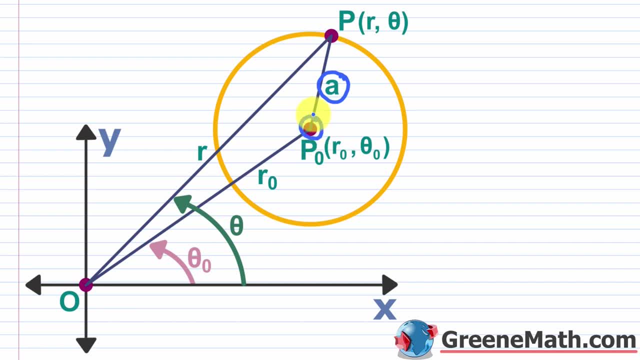 radius of this circle, okay, or the length from this guy right here, this point p sub zero to this guy right here, some point in the circle p. well, what i can do is i can use my law of cosines, right, because i have the length of this side here, which is r sub zero. i'll have the angle here, which is 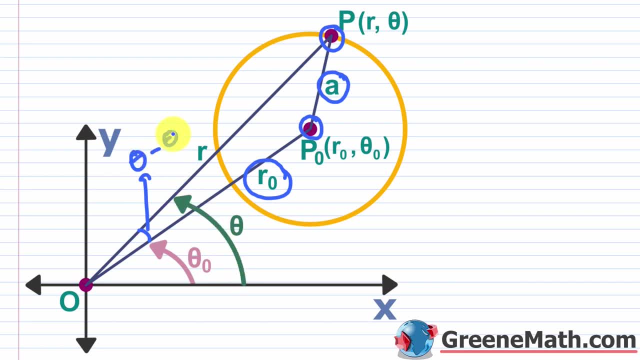 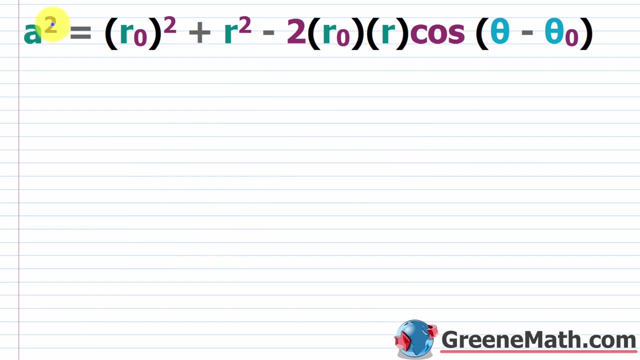 theta- okay, the bigger angle here- minus theta sub zero, which is the smaller angle here. okay. and then we'll have this side here, which is r, okay, so i have side angle side. so what i can do to get the length of this side a is set up my little law of cosines here. so a squared is equal. 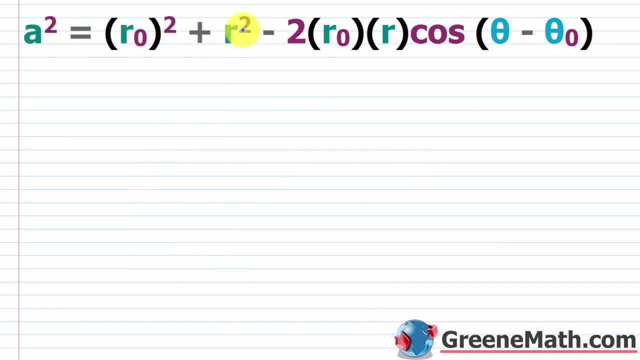 to you have your r sub zero being squared plus your r squared minus your two times r sub zero, times r times the cosine of theta minus theta sub zero. okay, now we're not going to actually work with this guy. what we're going to do is we're going to think about the first scenario. 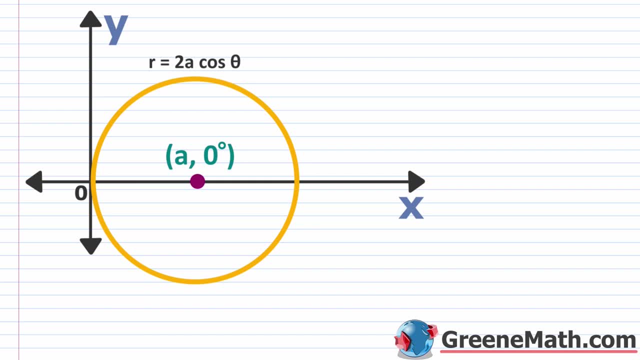 where our circle passes through the origin. okay, so now consider the fact that, again from the origin, if you called that, the point o to this guy right here, which we said was p sub zero, okay, the coordinates here now are a comma: zero degrees. okay, so your theta is going to be zero degrees. 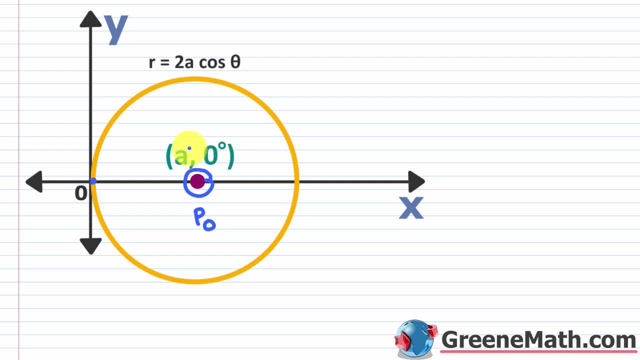 and your r sub zero is going to be a right, because the distance from the origin to the center is now going to be equal to the radius. so if we go back, this allows me to plug in for this r sub zero. i'm going to plug in an a and then i'm going to plug. 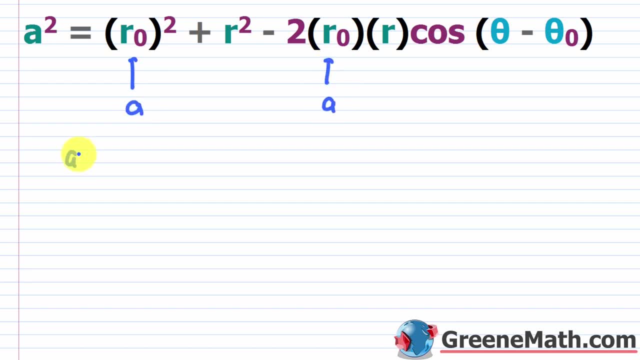 in an a okay, so we can simplify this. in this case we would have: a squared is equal to: you'd have a squared there plus r squared minus 2, a r times the cosine of. if i plug in a zero there, that's basically gone right. so i just have cosine of theta. so from here you can notice. 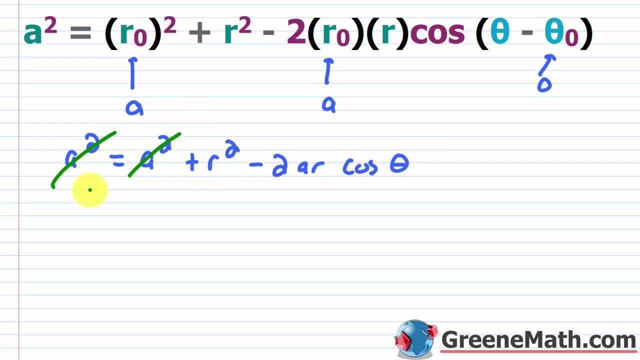 that this would cancel and you could move the r squared to the other side. so negative r squared is equal to negative 2 a r times the cosine of theta. i can multiply both sides by negative one, so essentially i just have: r squared equals 2 a r times the cosine of theta. now here's where. 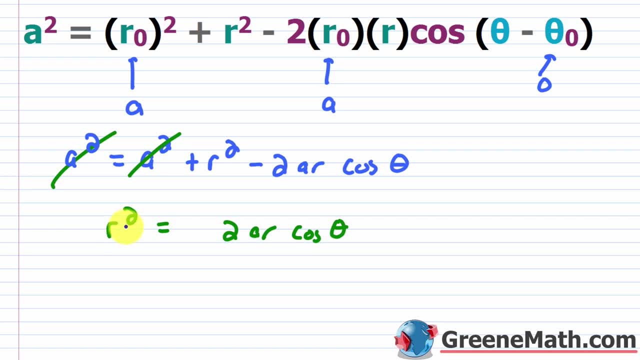 everybody gets a little bit lost. normally, if you have something squared, you take the square root of each side. in this case, we're going to divide both sides by r. okay, because r squared divided by r is r by definition, and so this is going to cancel here. so we're going to plug in for this. 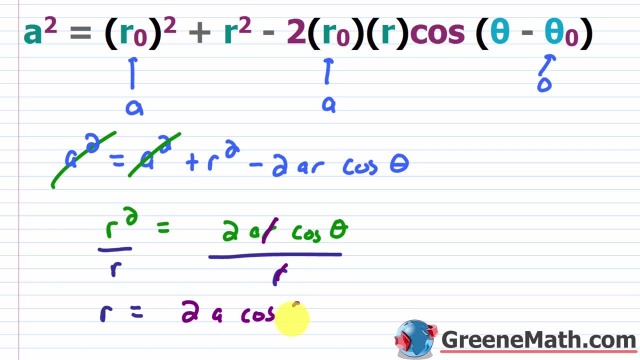 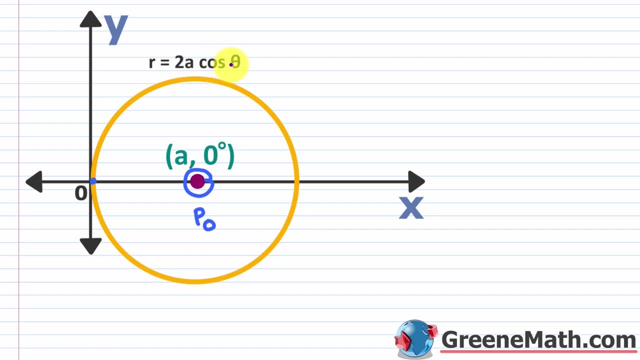 here, okay, and i'll have 2a times the cosine of theta, okay. so if you go back to this little diagram here, you'll see r equals 2a times the cosine of theta. so that's going to give me a circle that passes through the origin, that has a center on the x-axis, okay, and it's all based on. 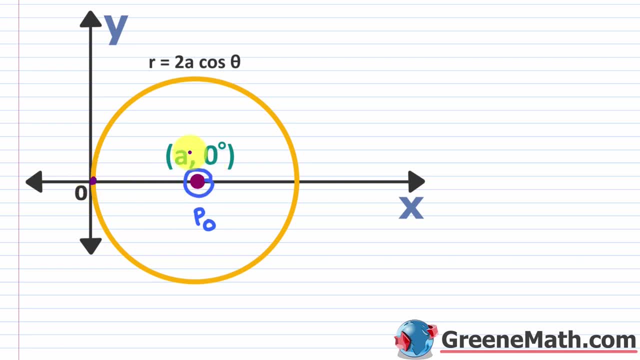 the fact that the distance from the origin to the center is given by this a here. okay, that's the radius of this circle. okay, now another way that you can derive this: if you don't like geometric definition or going through all that stuff, you can think about this in rectangular form. 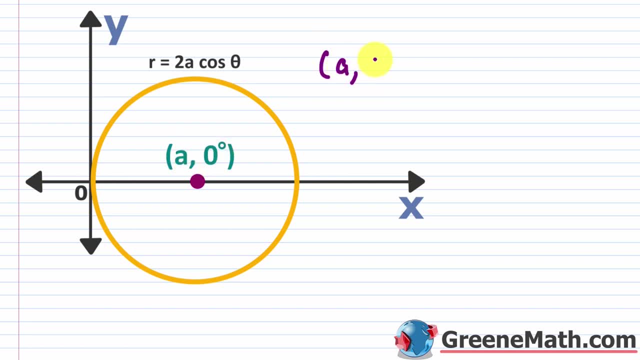 this a comma zero. degrees here would be a comma zero, and then it's easy to achieve this result. i would say, okay. well, i would say x minus a quantity squared plus. you would have y minus zero. quantity squared is equal to: in this case, the radius is a, so a squared. okay, let me go ahead. 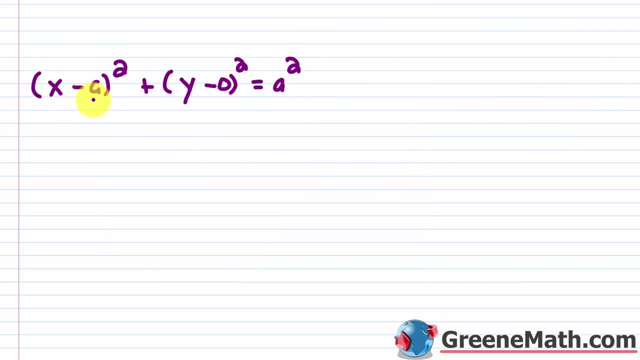 and copy this real quick. basically, what you'd want to do first is expand this. so you'd want to say: you have x squared minus 2ax plus a squared plus y minus zero is just y. so this is y squared, this equals a squared. you see again, you have the same thing on each side, so get. 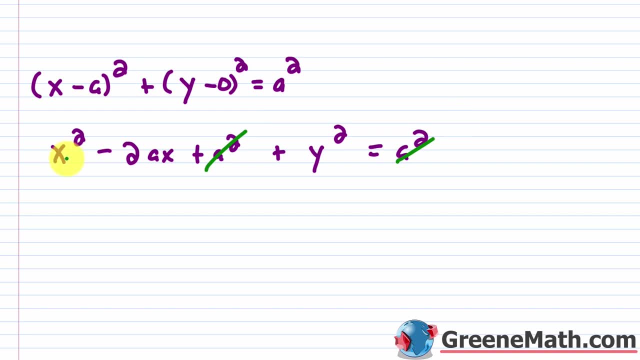 rid of this and this. that's gone. okay, so now i know if i have x squared plus y squared, again that's r squared. so you can rearrange things if you want to make that crystal clear. so x squared plus y squared and then minus 2ax would be equal to zero. okay, let me put this visibly, because some 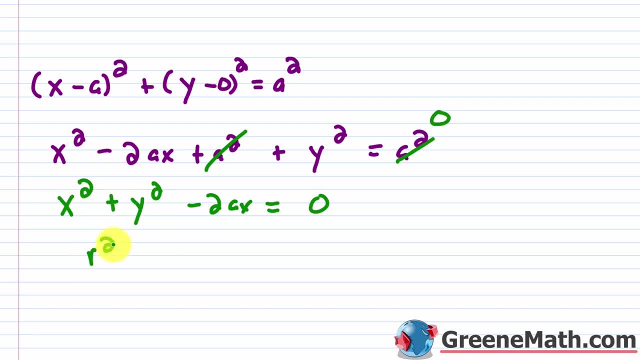 people get confused. cancel that over there. it's zero. so let me replace this with a square plus with r squared, and let me add 2ax to both sides, and now what you do is for x. remember, if you have x, you can always replace this with r times, cosine of theta. okay, so i'm going to put this as r times. 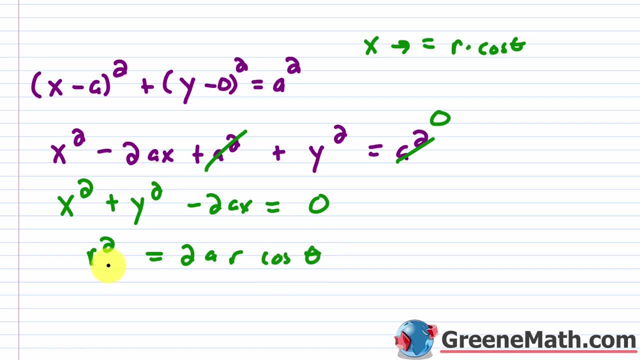 cosine of theta. and again, the confusing thing here is that, instead of taking the square root of each side, i'm going to divide both sides by r. that's something you just have to remember, okay. so what i'm going to do is basically cancel this with this, cancel this with this and say, let me scroll down. 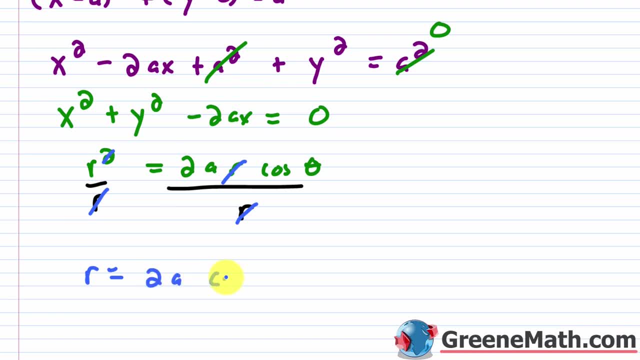 a little bit that i end up with a square root of each side, so i'm going to divide both sides by r is equal to 2a times the cosine of theta. okay, so if you see something in polar that looks like this, you can immediately convert it over and say it's x minus a squared. okay, that quantity squared then. 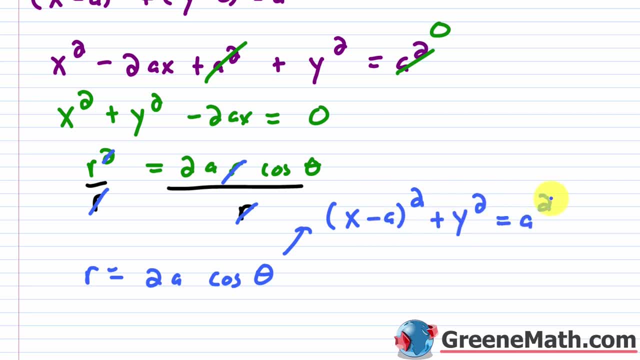 plus y squared is equal to a squared. okay, now converting back from this one to this one is a little bit more tricky. you have to check to make sure that everything matches up and i'll show you that in an example. okay, let's take a look at the first example. so we have x plus 2 quantity squared. 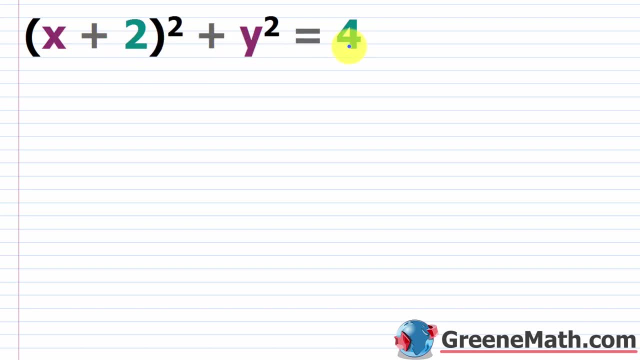 plus y squared, and then we have x plus 2 quantity squared, and then we have x plus 2 quantity squared equals 4.. okay, so the first thing is, if you want to make sure that this matches, the x minus a quantity squared plus y squared equals your a squared again. think about rewriting this. you have. 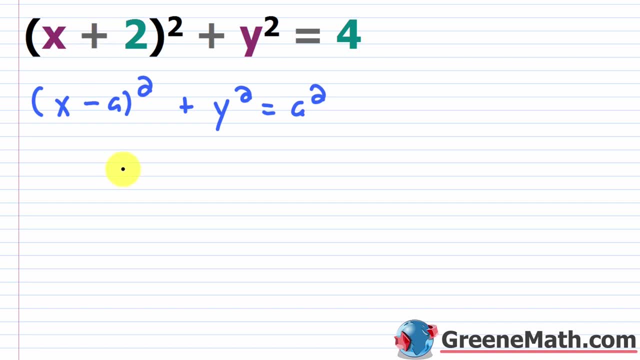 a plus here. how can i rewrite that? you want to do minus a negative? so you just want to match this and see if it works. so x minus a negative 2 quantity squared plus y squared is equal to you basically have negative 2 being squared. does this match? yes, now if you saw something like: let's: 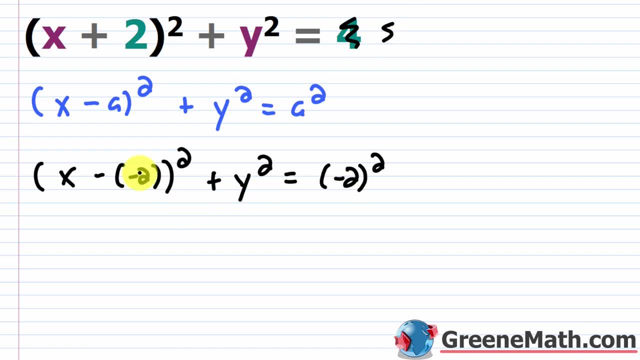 say this was 5, would this work out? no, because if i'm saying this is negative 2, well, negative 2 squared is not 5. okay, so you have to pay attention to this if you're going to use these shortcuts, okay, so what? i would? 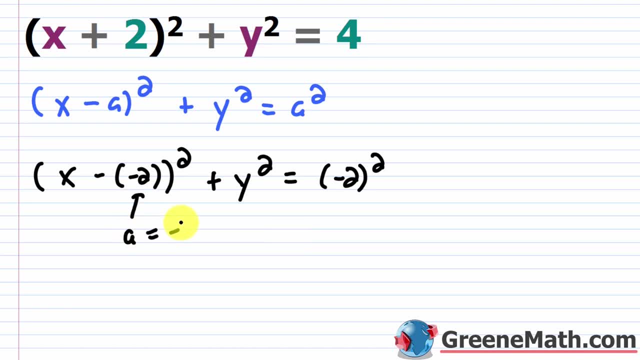 have here. is that a? my value for a is equal to negative 2, not positive 2, negative 2. so when i set this up, remember we said that r was equal to 2 multiplied by a, multiplied by the cosine of theta. okay, so here a is negative 2, so when i convert this over, i can just say that r is equal to 2. 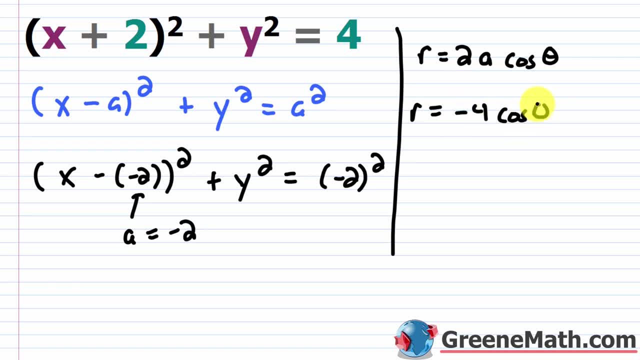 basically, 2 times negative, 2 is negative 4 times the cosine of theta. okay, once you do this a few times, it becomes very, very easy to convert these over. let me erase all this real quick and i'm just going to show you that you get the same thing if you do this the long way. so let me move this up. 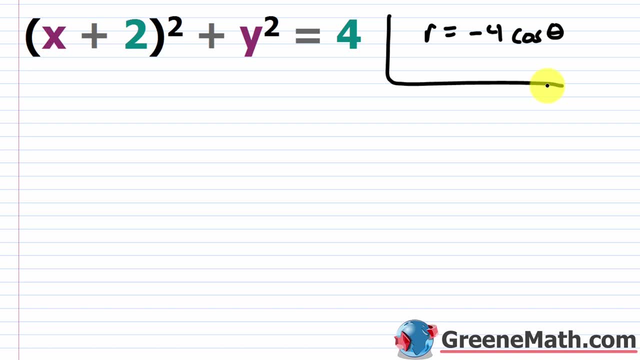 here. with these it's more of a time saver versus when you looked at the ones that were centered at the origin. so first i'm going to expand this. this would be x squared plus 2 times x times 2 would be 4x plus 4 plus y squared equals 4. okay, again you get this duplicate on each side of the equation. 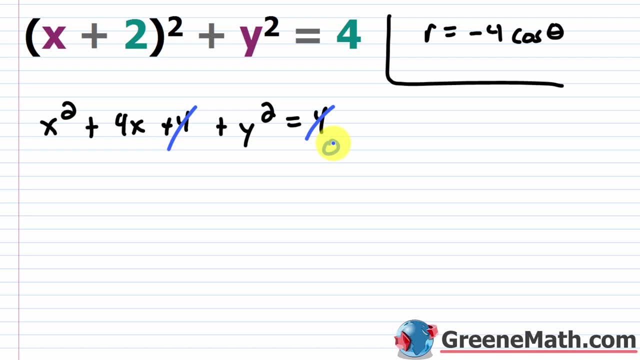 each side. so you get rid of that and this is 0. okay, so now you have x squared plus y squared. okay, that's going to be replaced with r squared plus 4x equals 0, okay, so from here, what i'm going to do is i'm going to replace this with r squared. i'm going to subtract 4x away from each side, okay. 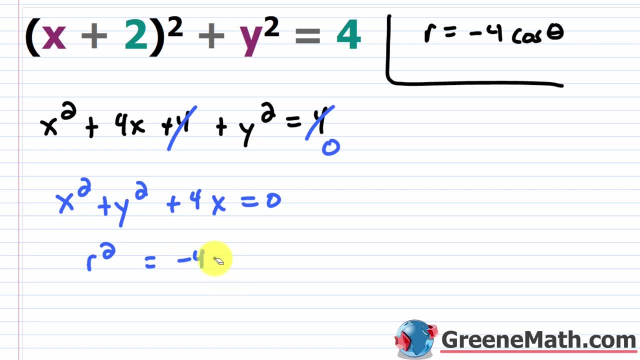 and all i really need to do now is replace x with r times cosine of theta. so r times cosine of theta. and again, this is the key- we're going to divide both sides by r. okay, do not take the square root of each side. you want to divide both sides by r, so this is going to give me that r is equal to, again, this: 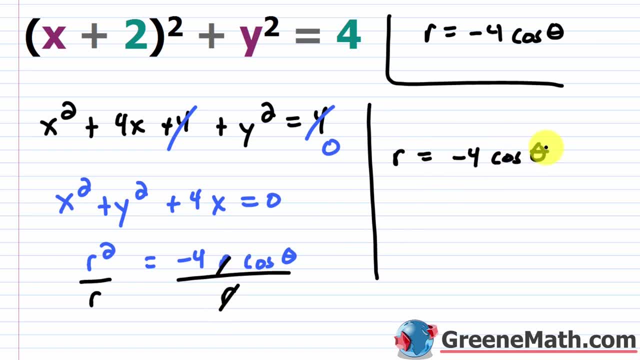 cancels negative 4 times the cosine of theta. so however you want to do this, you're going to get the same answer. okay, just make sure that if you're using the shortcut, that things match up. if this was 5 or 6 or 10 or something like that, this would not work. this would not be a circle that goes to. 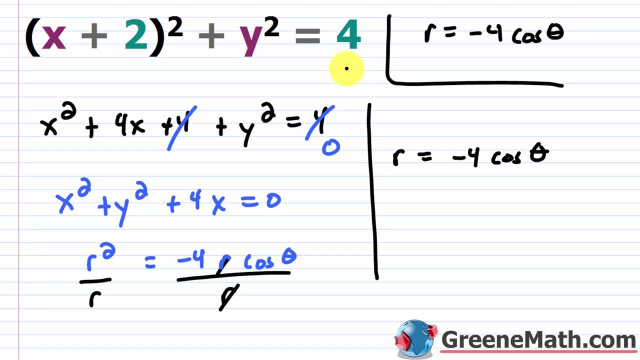 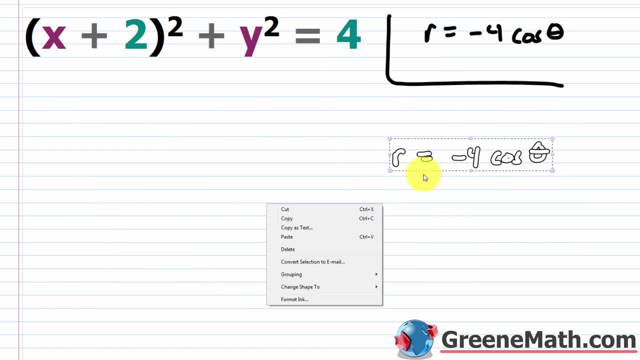 the origin that is centered on the x-axis. this is where this formula works. now, if you wanted to graph this, this is a lot more difficult, or a lot more challenging, i would say- versus when you worked with graphing a circle on the rectangular plane. the reason is, when you work on the rectangular plane, you can plot your center and then from your 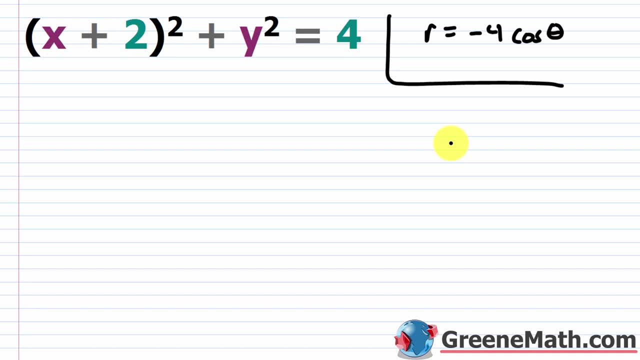 radius. you can just move up by that amount, to the right by that amount, down by the amount and then left by that amount. then you can draw your circle right. you're done with this guy. you basically have to make some points, okay? so let me put an r value and then a theta value here, and you just have to. 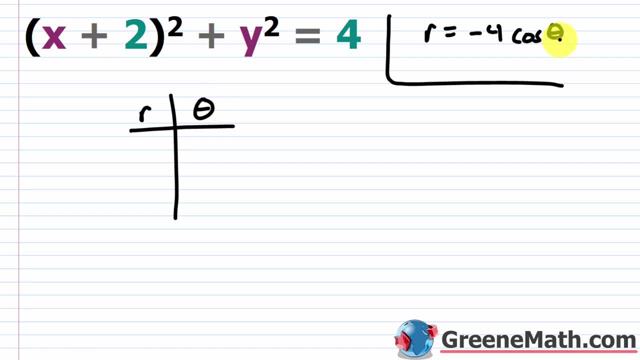 use some logic, Okay. So, first off, I'm always going to try the cosine of zero. I know that's one, So let me put zero. I'll do this in terms of degrees, So zero degrees, Okay. So the cosine of zero degrees is: 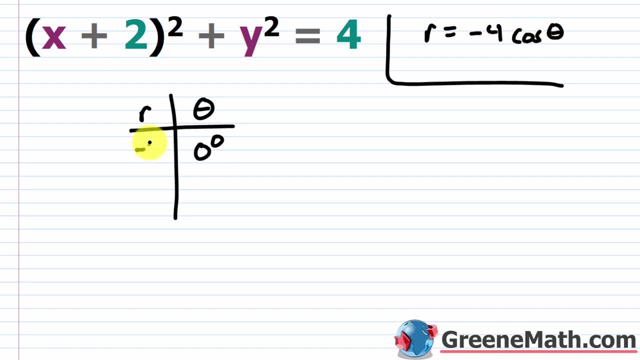 going to be one negative four multiplied by one would be negative four. Okay, So one point would be negative. four comma: zero degrees. Another point: I always try 90 degrees because I know cosine of 90 degrees is zero. So that would be negative four times zero, which would be zero. 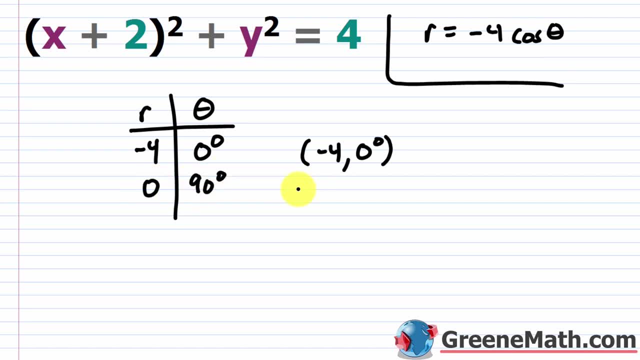 So if I put 90 degrees I would get zero. Okay. So basically this point would be zero comma 90 degrees. That's just going to be on the pole. Okay, Then other things you could do. if you had this as a half right, Negative four times a half would give you negative two. If you want something. 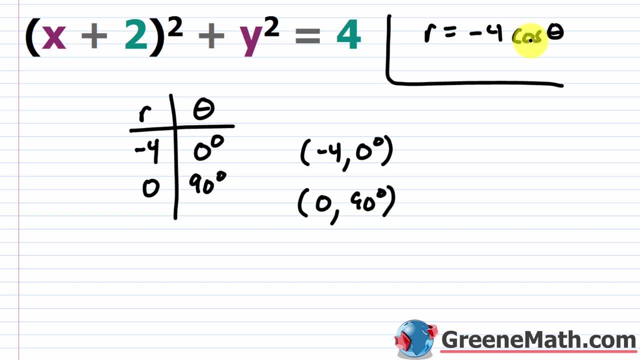 that's positive for the R, then you're looking for negative a half. Okay, So you know that cosine of 60 degrees is a half, but if you want it to be negative it's got to be in quadrants two or three. 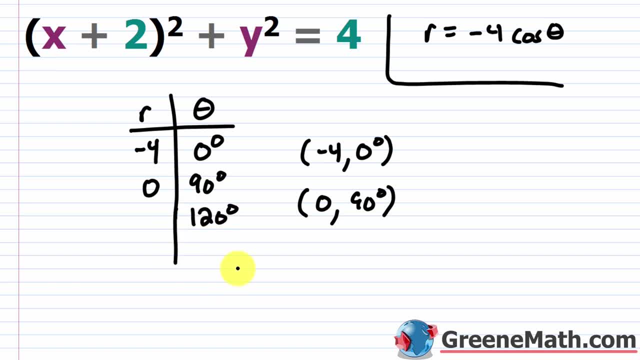 So you'd want something like 120 degrees, Okay, Which is a 60 degree reference angle in quadrant two, Or 240 degrees, which has a 60 degree reference angle in quadrant three. So now I would say: okay, well, the cosine of either 120 degrees or 240 degrees is negative, a half negative, four times. 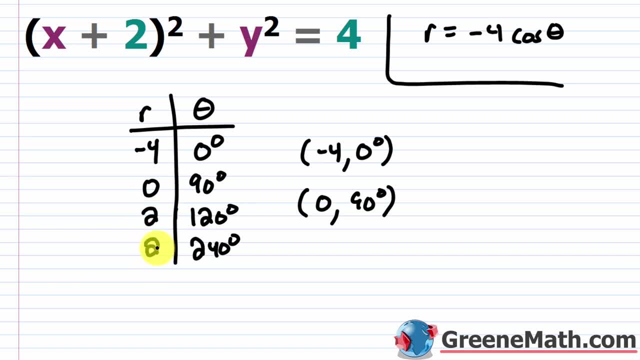 negative a half is two. Okay, So this is two, and this is two. So there's two more points. So you have two comma 120 degrees, and then you have two comma 240 degrees. Okay, So let me grab these real. 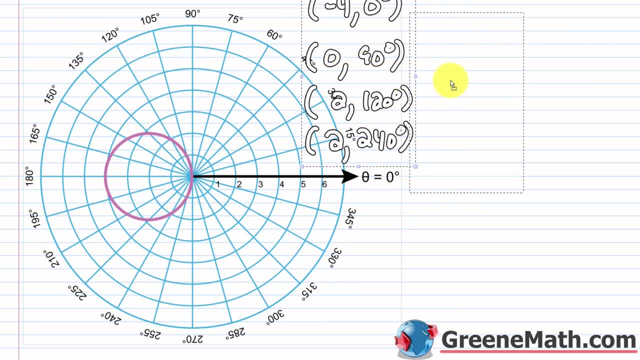 quick, Let me copy them All, right? So obviously I've already graphed this guy, Okay, But I just want to show you how to do that. So I'm going to go ahead, and I'm going to go ahead, and I'm going. 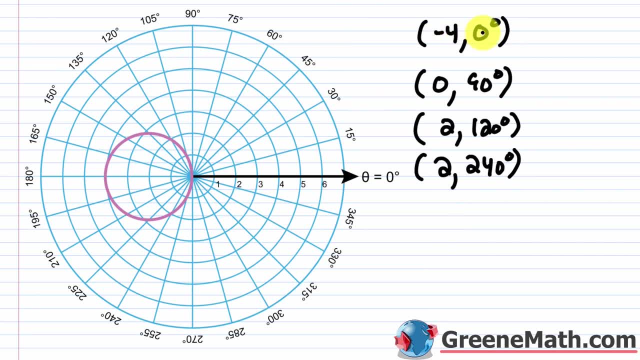 to show you how you can do this. So we have negative four comma zero degrees. I would convert this and say this is four comma 180 degrees, just to make it simpler. And essentially that would be what. So I would go out to a circle with a radius of four and then swing around to 180 degrees. So 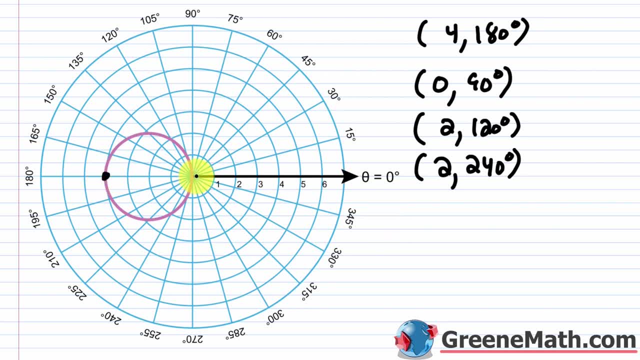 right there, and then zero comma, 90 degrees. It doesn't matter the angle. If you have a radius of zero, you're not going anywhere, Right? So from the pole you're stuck right. It doesn't matter which way I'm looking or turning or orienting myself, I'm just going to be on the pole, Okay. 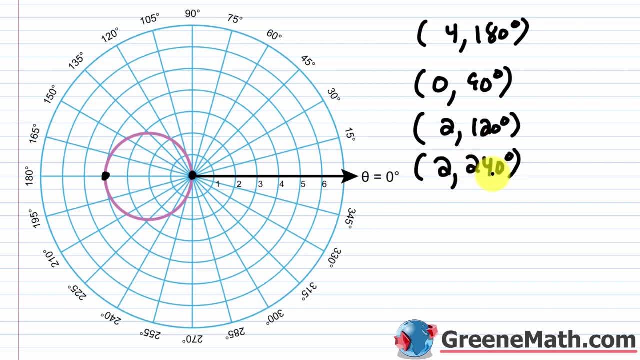 Then two comma 120 degrees, or two comma 240 degrees. So in each case you're going out to a circle with a radius of two, and then I'm going to swing around to 120 degrees, And then I'm going to swing around to 240 degrees. Okay, So from those four points, that's enough to sketch the. 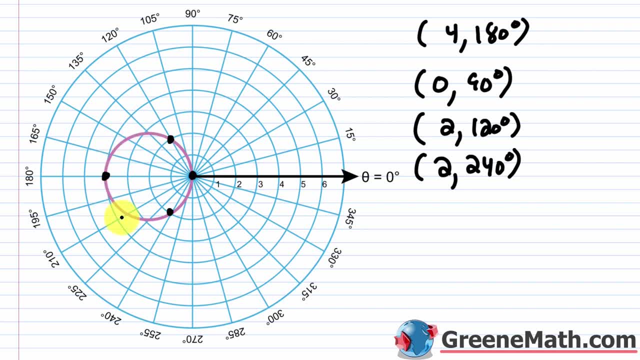 graph of that circle. If you're using a computer, obviously it's going to be perfect, but if you're doing it freehand, just notate your little points there So you can show the teacher you found some points and then sketch the circle the best way that you can. Okay, Let's look at another example. 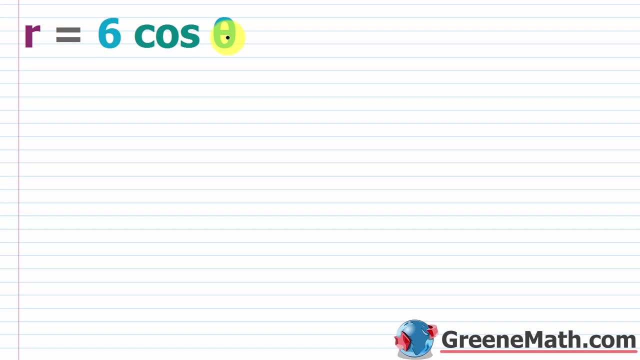 We're given this guy in polar form. So R equals six times cosine of theta. Now, be very, very careful When you look at the formula. remember it's R is equal to two A times the cosine of theta. Six is not A. Okay, You have to do some extra work here. You would say that. okay, well, 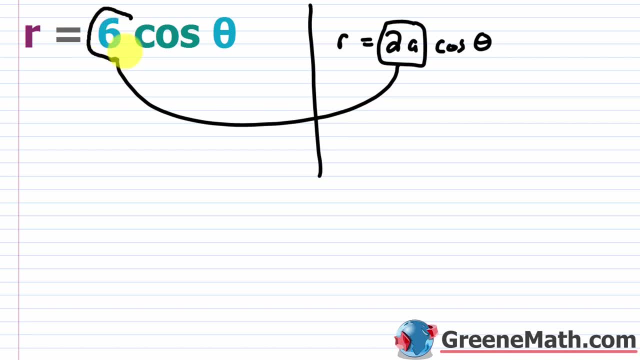 this guy right here is equal to this guy right here. Okay, So two A is equal to six, which means if you divide both sides by two, A is equal to three. Okay, So, once you know that A equals three, converting this over is pretty quick, right? So let me write here that A equals three. What I would 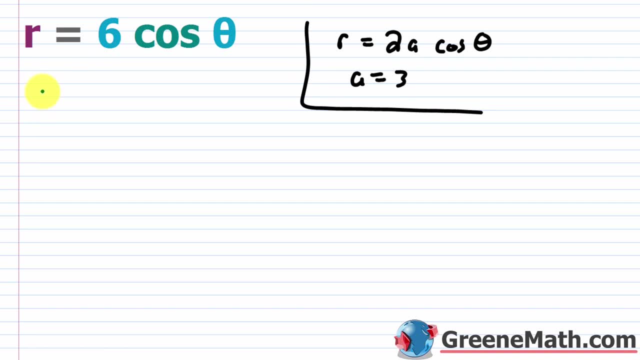 do, I would say, okay, well, I know that we have this form of R equals two A times the cosine of theta, and this goes to: X minus A quantity squared plus Y squared is equal to A squared. Okay, We know that. So here I'm just going to plug in. Everywhere I see an A, I'm just going to put a. 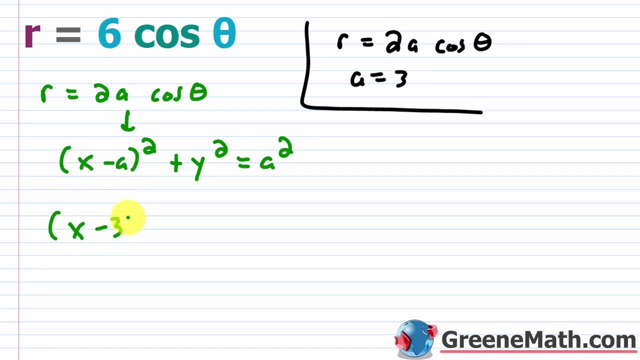 three. So this would convert itself over to X minus three. quantity squared plus Y squared is equal to three being squared. So I'm going to put a three. So I'm going to put a three. So I'm going to put a three. So that's the quick way to do it. But again you've got to make sure that you match. 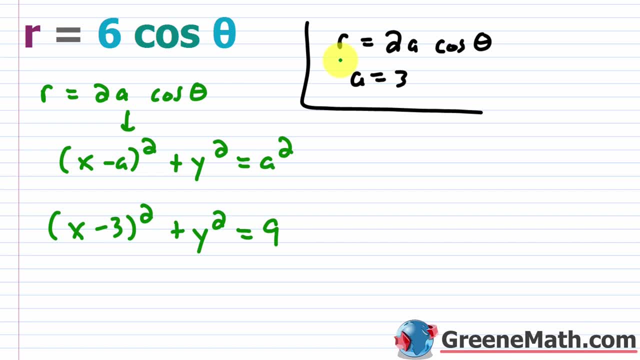 things up correctly. If you want to ensure against the mistake, then you can always do this the long way. So what I would do here is I would multiply both sides by R, So that gives me R squared Okay, Which we can replace, And it gives me six times R, times cosine of theta. Remember whenever I see. 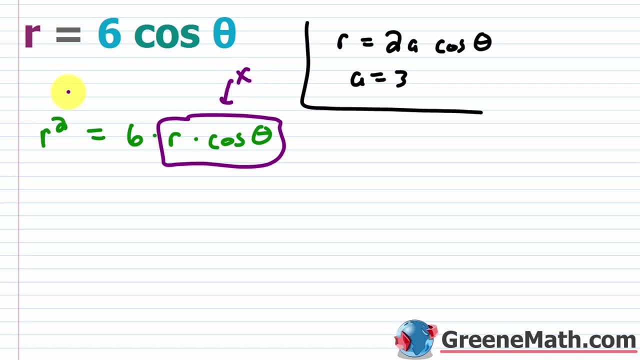 R times. cosine of theta. I can replace that with X, And whenever I see R squared, I can replace that with X squared plus Y squared. Okay, So I'm going to have X squared plus Y squared is equal to six X. What I'm going to do is move this over to the other side, So I'll 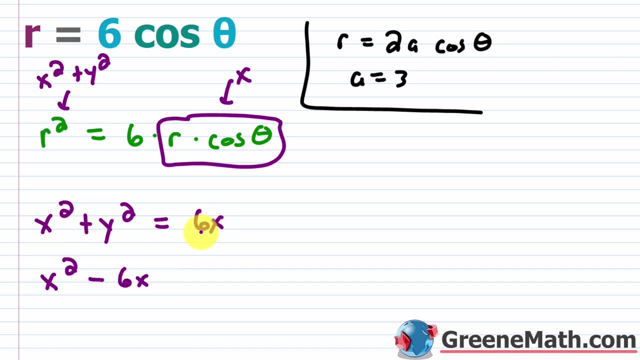 say I have X squared, And then I'll say minus six X, because I'm subtracting this away from each side, And then I'm going to leave a space because we're going to need to complete the square. then plus Y squared, and this equals zero. Okay, So let me get rid of all of this. 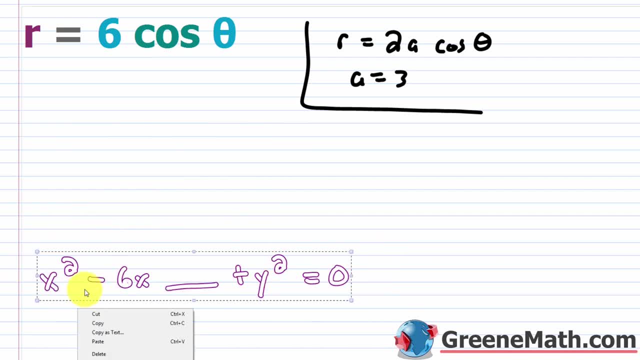 just so I have a lot of room to work. get rid of this And let's move this up. So maybe it's been a while since you completed the square, But remember, what you want to do is you want to look at this coefficient right here. In this case it's negative six. It's always the one that's. 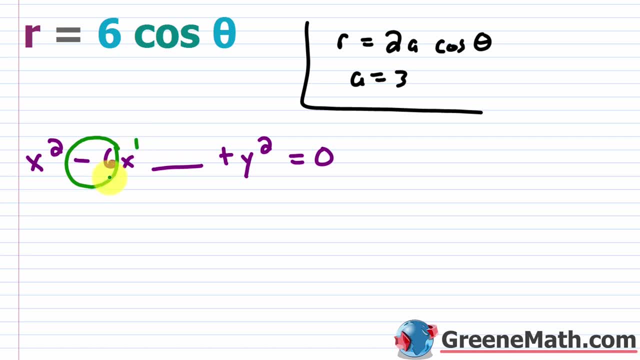 on the variable to the first power. Okay, so X, the first power, So negative six. you want to cut it in half or multiply by half, And then you want to square the result. Okay, so negative six divided by two, or negative six times a half, is going to be negative three. So then negative three squared. 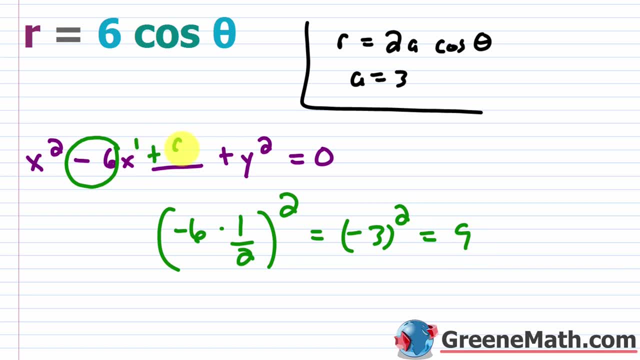 is equal to nine. Okay, so from here, I'm going to add nine to both sides to make this legal, can't just add it to one, And essentially what I'm going to have here is a perfect square trinomial on the left hand side. Okay, I don't need to do anything here, because this is Y squared. 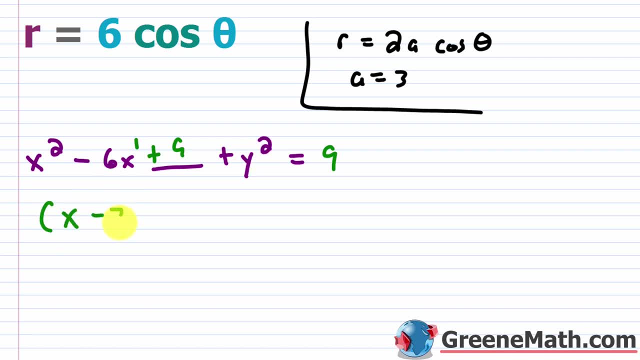 can't do anything with that. So with this one I'm going to go okay, x minus three, quantity squared is how you'd factor that. then plus Y squared is equal to not okay. And again, it's easier if you use the formula. But sometimes if 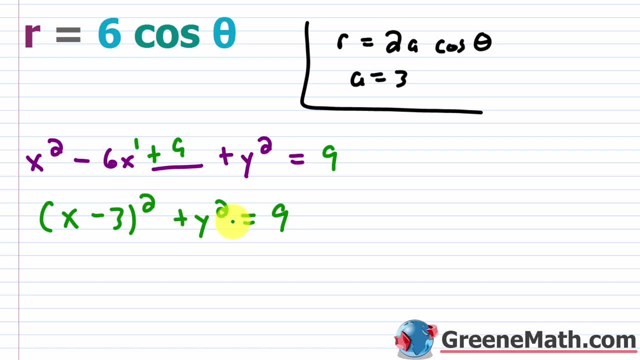 you're not super familiar with how to work with the formula, you might as well just go through this to guard against any mistakes. Okay so let me erase and let's talk about graphing this guy. So again, I would put some points here. So R and then theta. Okay, So if I'm thinking about some, 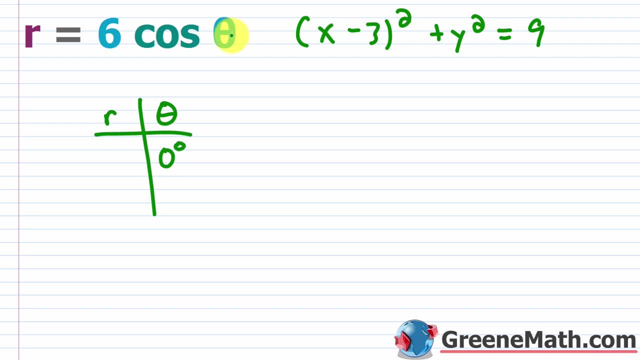 thetas. I'm always going to go with zero degrees. cosine of zero degrees is one, so R would be six. Then if I think about, let's go ahead and do 90 degrees, okay. cosine of 90 degrees, I know, is zero. six times zero is zero, So R is zero. Okay, so it's gonna be at the pole Again. 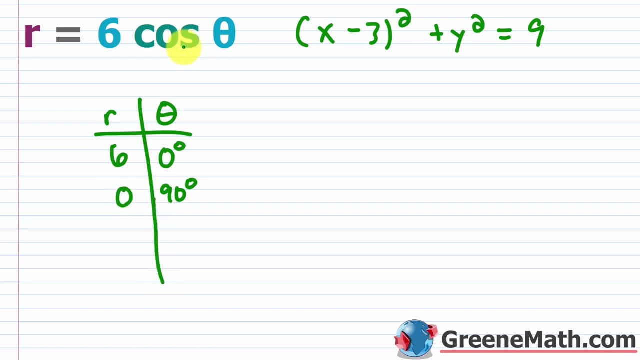 let me think about the cosine of 60 degrees is going to be a half, right. So six times a half is three. Okay, I'm trying to get some whole number of values here, So I could do 60 degrees. okay, that would give me three. And then also cosine is positive. 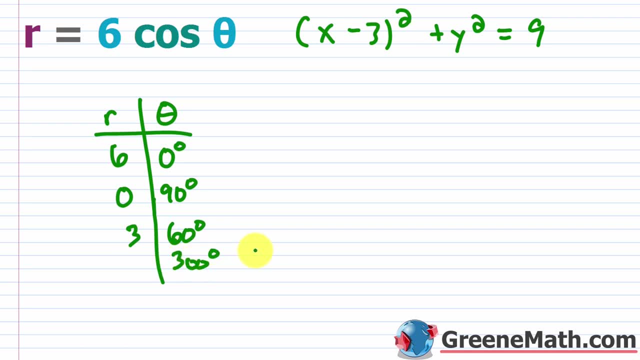 quadrant four also, so I could do 300 degrees. that has a 60 degree reference angle, And I'm going to get three here as well. Okay, so this would give me six comma zero degrees. this would give me zero comma 90 degrees. this would give me three comma 60 degrees, And this would give me 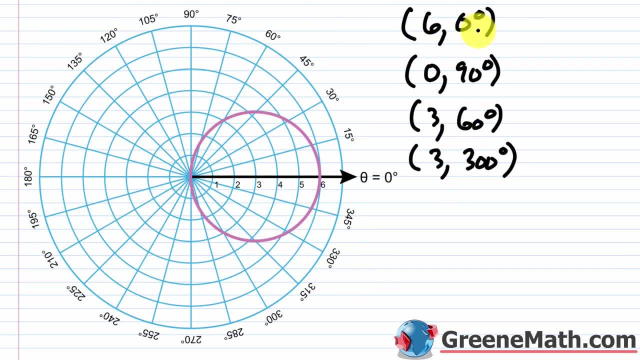 three comma 300 degrees. And again, if I want six comma zero degrees, well, basically, from the pole, I'm just walking to the right, six units, right, so I'm gonna be right there. And then zero comma 90 degrees, again, if the radius is zero, I'm not moving off the pole. And then three comma. 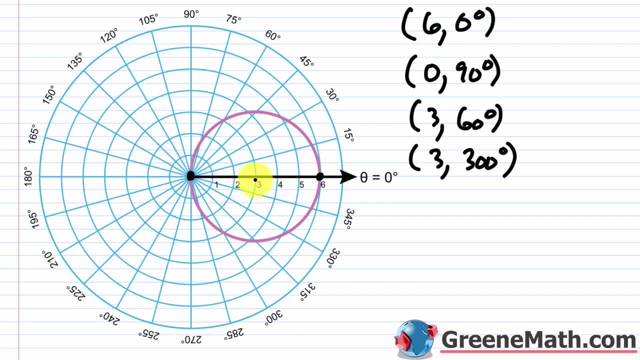 60 degrees. again, I'm going to go out to a circle with a radius of three and then swing around to 60 degrees. So that's right there. Then three comma 300 degrees, circle with a race of three, And I'm 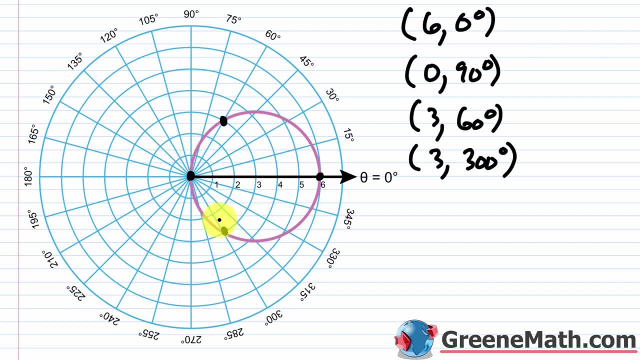 gonna swing all the way around to this: 300 degrees right here And again. these are enough points here to where you can plot them and then sketch a nice little circle through the points. Again, doesn't have to be perfect, just notate your points So you teach. you can see that, Alright. so 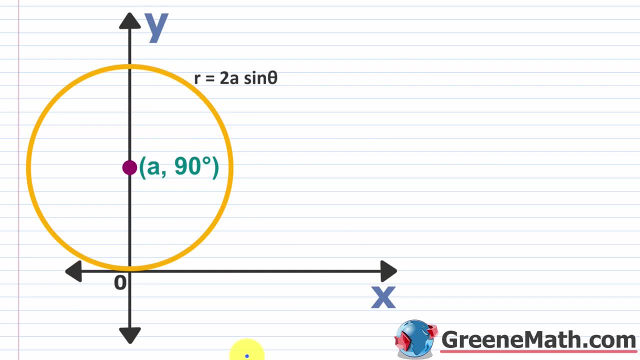 another common occurrence is going to be a problem where the center is on the y axis and the circle is going to pass through the origin, So in other words, from the origin, which is a point on the circle, to our center. okay is. 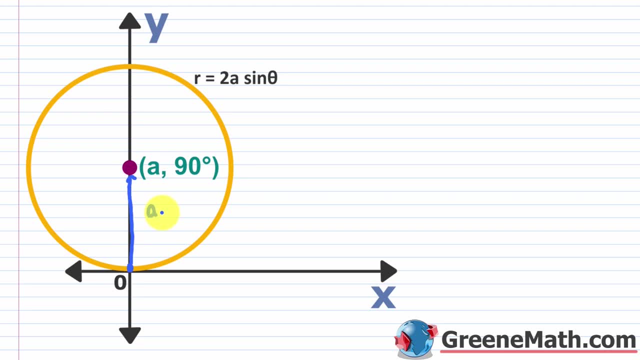 going to be a distance of a, so that's going to be the race, okay, So the sensor occurs at a comma. in this case could be a 90 degree angle, right, If I'm thinking about this, this is a right angle. 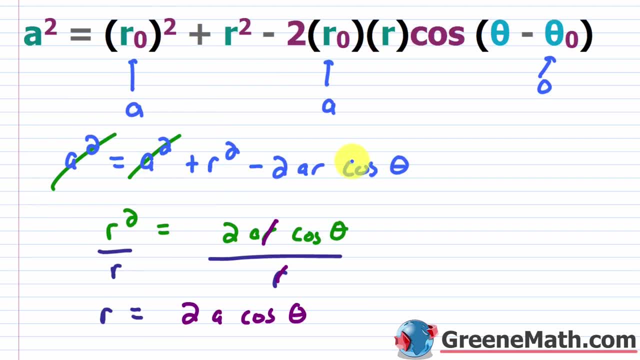 So it's 90 degrees, And essentially, if I wanted to come back up here, I would change only a few things. So let me get rid of this. And now this would be 90 degrees that I'm plugging in here. So 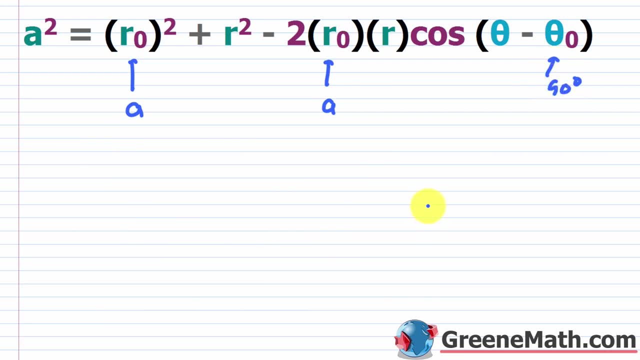 that's a change, Okay, So first let's go through and do the cosine of we'd have theta minus 90 degrees. Remember, this is going to be your difference identity for cosine. So it's the cosine of the first guy, which is theta times the cosine. 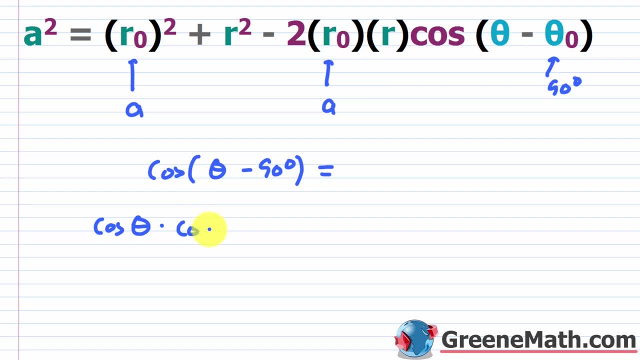 of the second guy, which is 90 degrees. Let me write that a little bit better. So what is the cosine of 90 degrees? we know that's going to be zero, so you just get rid of it, right, But I'll. 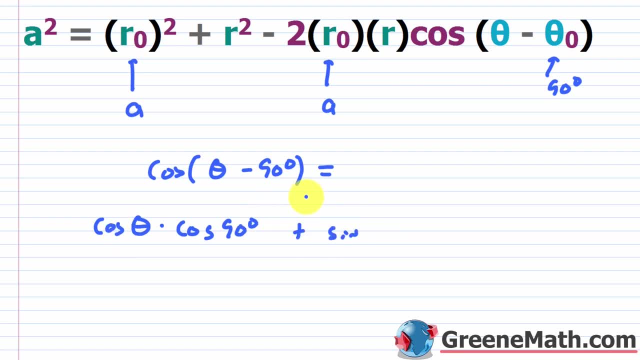 leave it right now. So, plus, then you're gonna have the sine of the first guy, which is theta, and then times the sine of the second guy, which is 90 degrees. Okay, So we know this is gone And we know that the sine of 90 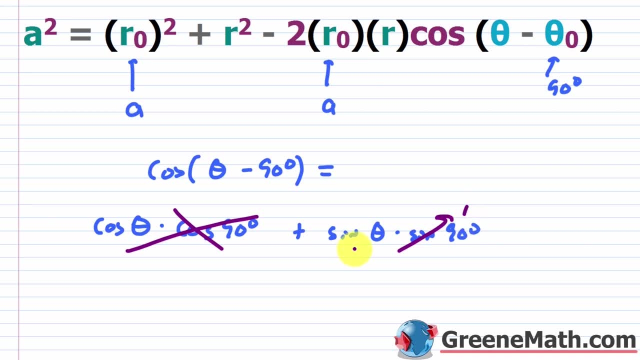 degrees is one, you'd say that's one. So, basically, this is gonna end up being sine of theta, Okay, So what I'm going to have here? I know that this would be a squared and this would be a squared, So get. 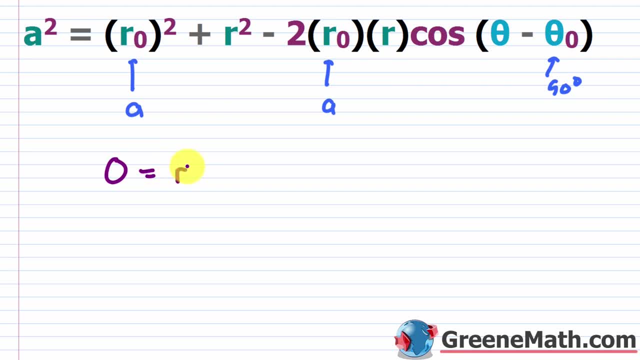 rid of it. I'm just going to say that I would have. zero is equal to r squared minus two, a r. Okay, Instead of cosine of theta minus 90 degrees. we know that this is the sine of theta, So sine of theta. 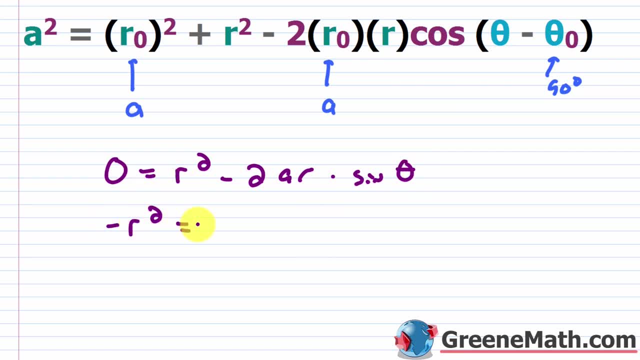 Okay, Let me move this over. So negative r squared is equal to negative two a r, and then times the sine of theta. let's get rid of this, And I'm actually going to get rid of this right here. Okay, Let's. 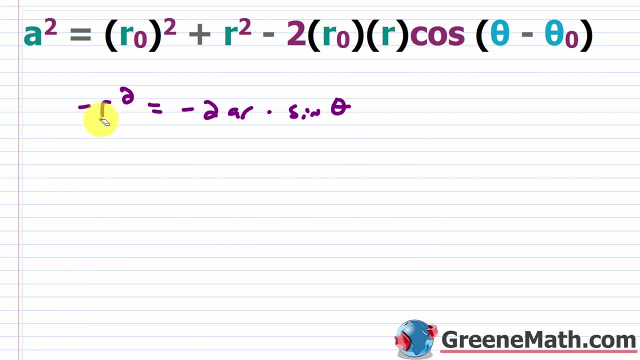 move this up like this, And I'm going to multiply both sides by negative one, get rid of the negatives And essentially, from here, I'm just going to divide both sides by r, okay, like I keep doing. So what's going to happen is this is going to cancel with this. this is going to cancel with. 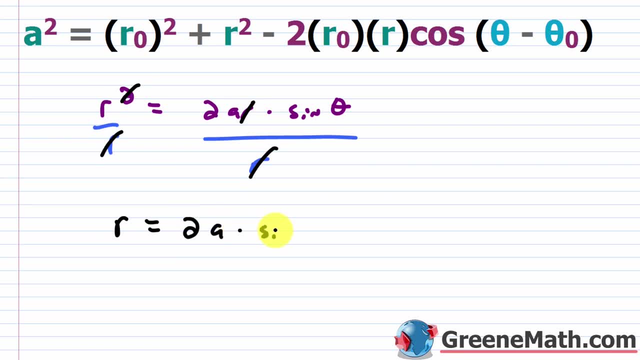 this and you get: r is equal to two a times the sine of theta. Okay, So if r equals two a times the cosine of theta, it's going to pass through the origin and it's going to be centered on the x axis. If r equals two a times the sine of theta, it's going to pass. 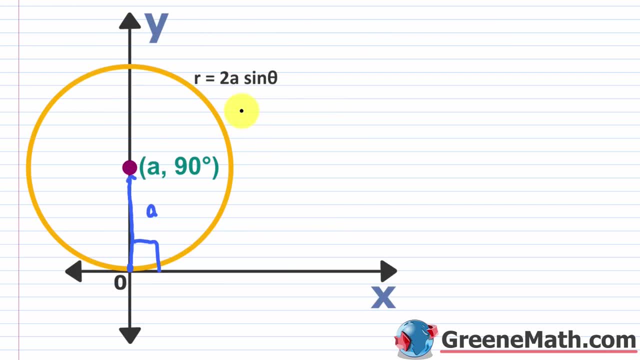 through the origin. it's going to be centered on the y axis. Again. if we go back to this guy, get a race, this. If you think about these coordinates here in rectangular, this would be what it would be: zero. that's the x location and then the y location would be a. So now, if I 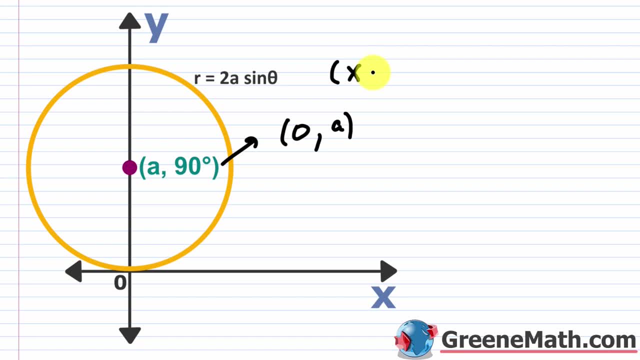 think about this in rectangular. you would have x minus zero. quantity squared plus, you would have y minus a. quantity squared is equal to. again, the radius here is a. the distance from the origin or a point on the circle to the center is going to be given by a. So I can. 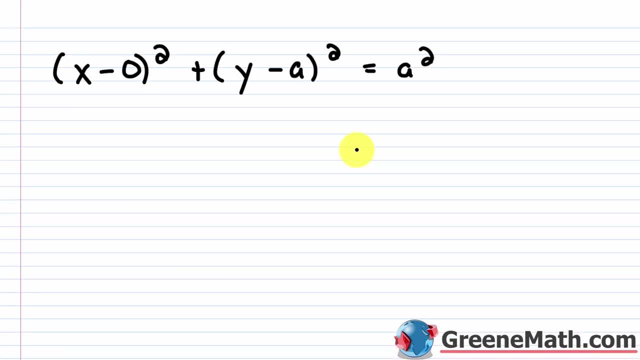 say: this is a squared, Okay, So let me grab this real quick. So what I'll do from here? I'm going to write this as just x squared, because obviously x minus zero is just x, Then plus, I'm going to. 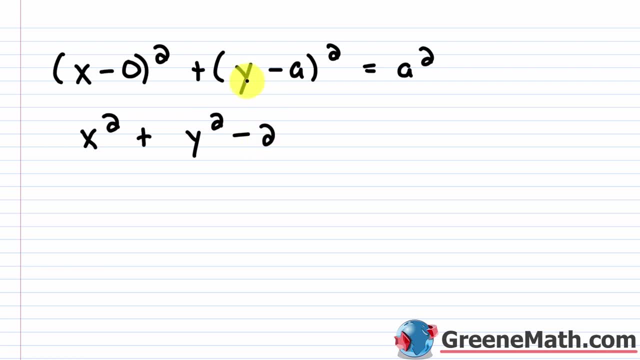 expand this So this will be y squared minus two times y times a. So let's write: minus two times a plus a being squared And this equals a squared. So you'll notice that again I could subtract a squared away from each side. So basically, let's just line this out, put a zero here, Okay, And 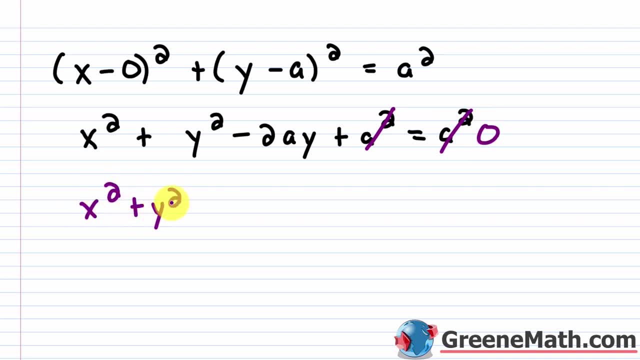 then from here I'd have x squared plus y squared. We know we can replace that with r squared. Let's do that in a second. I'm going to say: this equals to: I'm going to move this over here, So I'm going. 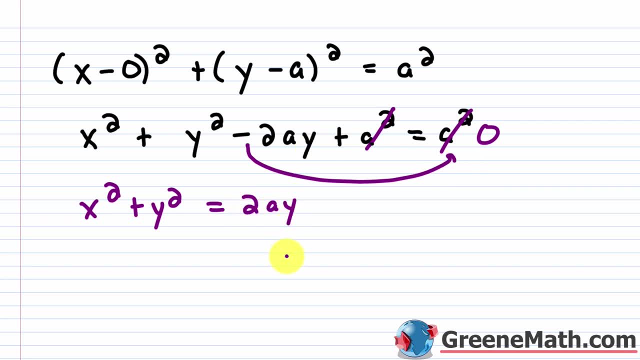 to add two a y to both sides. I'm going to put two a y like this: And now all I need to do is take x squared plus y squared, replace that with r squared, And then I'm going to add two a y to both sides. 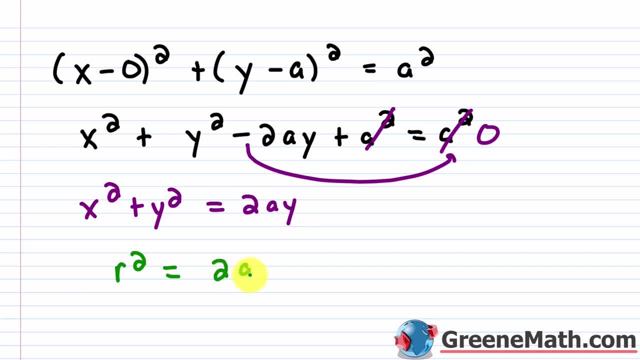 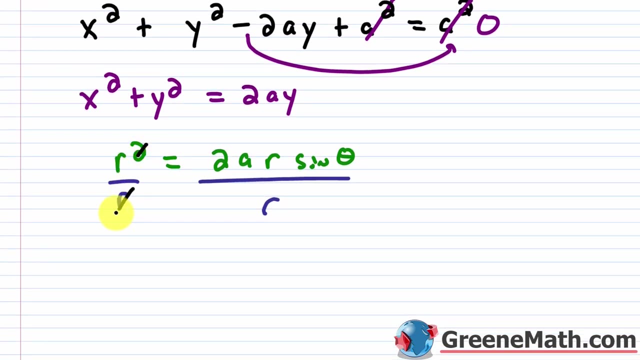 And then the two a- y. I'm going to put two a and replace y with r. times the sine of theta, Okay. And then for the last step, I'm just going to divide both sides by r. So let me scroll down and get a little bit of room going here, And all we're going to do is just cancel one of these with. 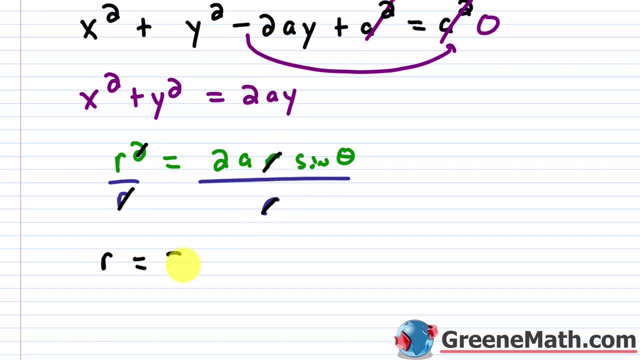 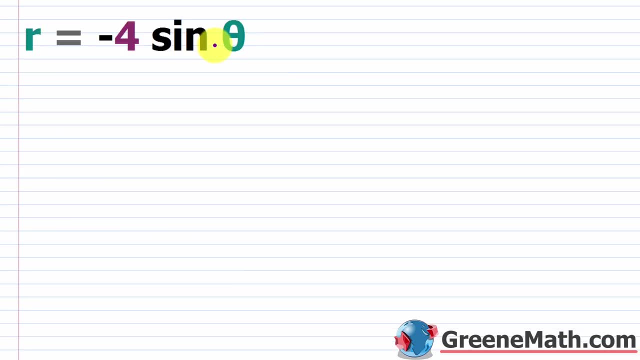 this and this with this, And I'll say: r is equal to my two a multiplied by my sine of theta. Okay, Let me make that s a little bit more clear, All right? So for our example we'll look at: r equals negative four times the sine of theta. So again, if you see something that looks like r, 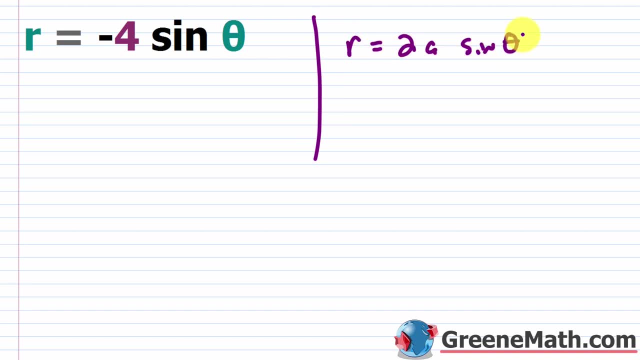 equals two a times the sine of theta. this guy's going to pass through the origin and it's going to be centered on the y-axis. Okay, So again, don't just take negative four, two a, this part right here. let me do this in a different color, so this is clear. So two a is going to be equal to: 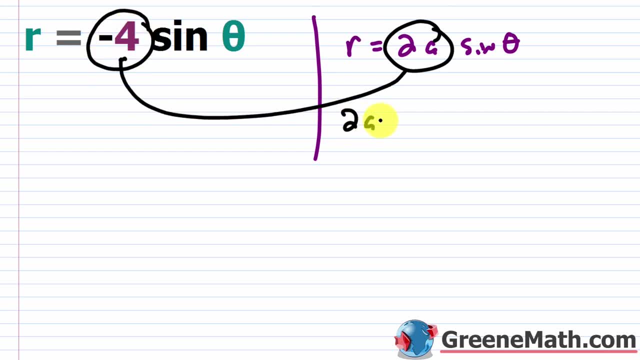 negative four. So that means that basically you have two. a equals negative four. divide both sides by two: a equals negative two. Okay, So make sure you're understanding that, Understand what you're plugging in. So if a equals negative two and you want to plug into 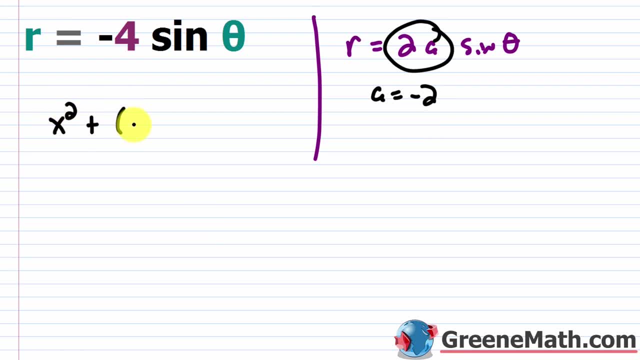 that formula. So we're going to have x squared plus, you'll have your quantity, y minus a. In this case it's minus a negative two, Okay, And that's going to end up being y plus two, but I'll change that in a moment. So this is squared and this equals the radius which is a being squared. 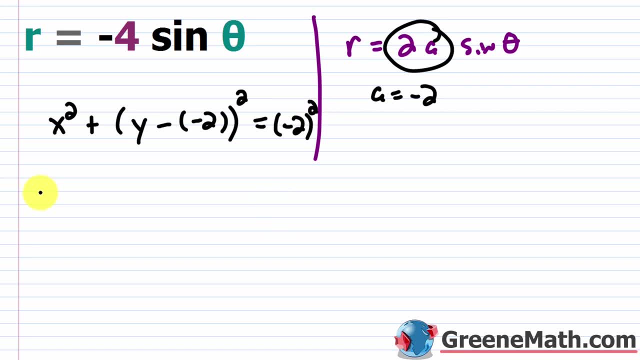 So you'd have negative two being squared. Okay, So this ends up being x squared plus. you'd have y plus two. Okay, Quantity squared is equal to four. Okay, Converting it over to rectangular using our little formula. Now, if you don't want to do, 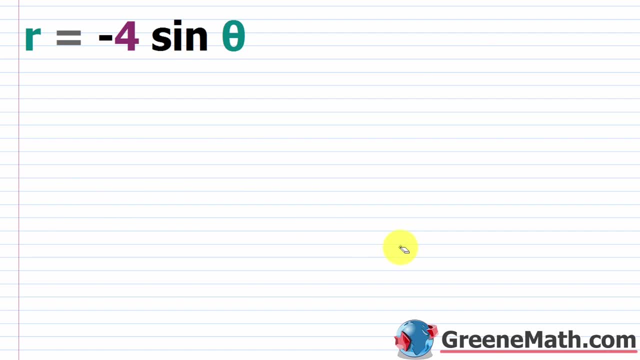 this or you're not comfortable with this. again, it's fine, It's no big deal, You can always do this the long way, Okay, So for this one I would multiply both sides by r, So you get r squared is. 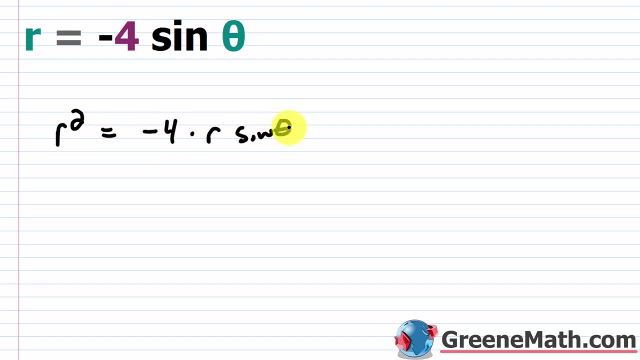 equal to negative four and then times r times the sine of theta. If you have r times sine of theta, that's y, Okay, So just go ahead and replace that with y. Replace r squared. I'm not going to have room for this, but you want to replace r squared with x squared plus y squared, So this is x squared. 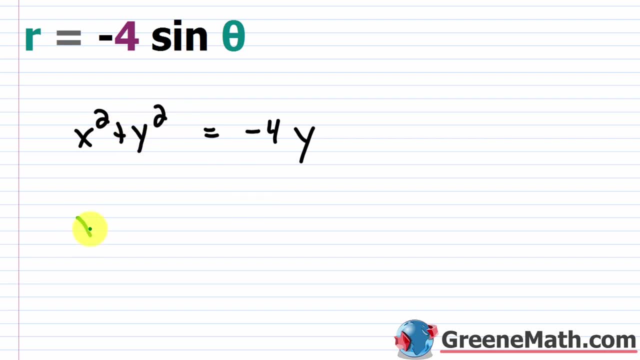 and again, you're just going to move things over and complete the square. That's all you need to do. So this is x squared, plus I'm going to go ahead and say this is y squared, And then I'm going to. 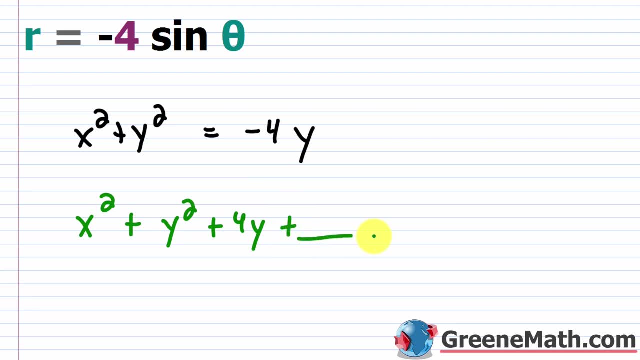 add four y to both sides, Okay, And I'm also going to leave a space here and I'll put equal zero right, Because I added four y to both sides. So here I need to cut four and a half. So that'd be. 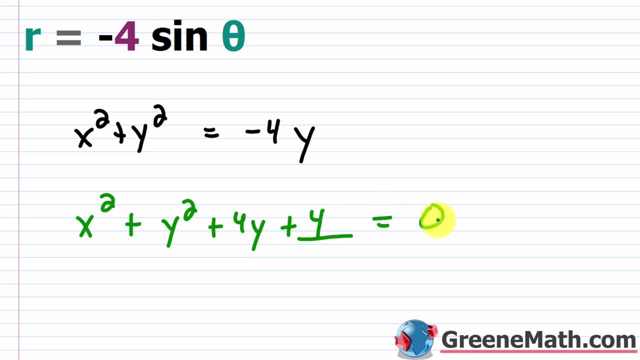 two and then squared. I get back to four Now, because I added it over here. I've got to add it over here. So this equation becomes this: To get rid of all this: Okay, So I'm going to go y plus two quantity squared, and then this equals four. Okay, So this equals four. So it's. 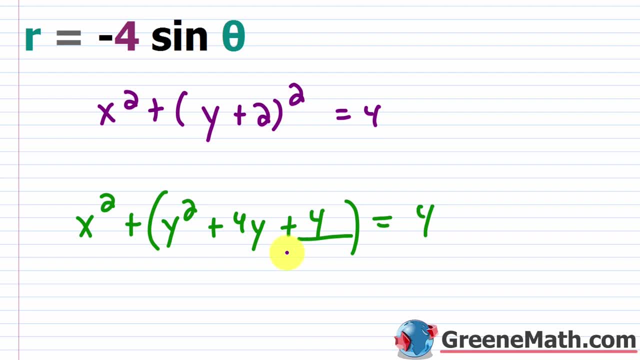 not that bad overall if you're really good with going through the steps. on this, I like to use the formula: If I see something immediately, it's just a lot quicker for me, But if you want to guard against errors, this is a surefire way to do it every time. So let's think about graphing this. 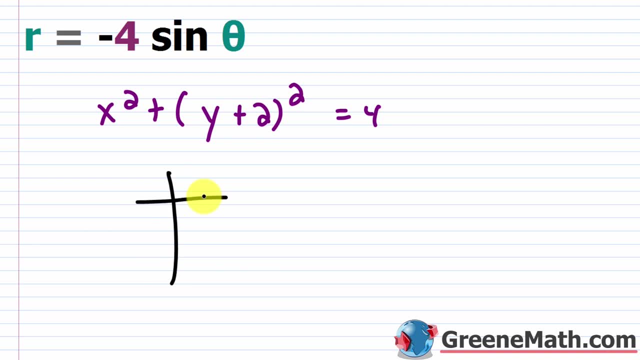 now, Again, what I want to do is get some points, So I'm going to put r and then theta, So the first one that I'm going to do. again, I always do zero degrees, So I know that the sine. 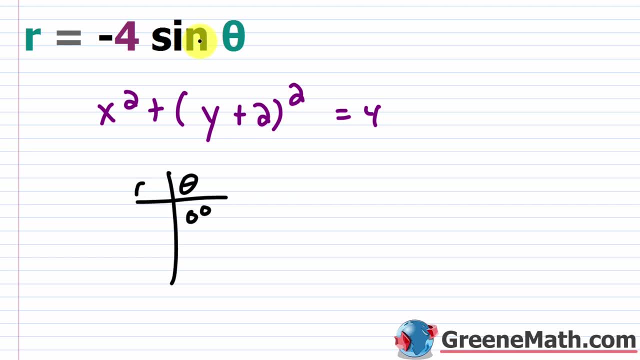 of zero degrees is zero. So negative four times zero is zero. Okay. And then if I did, let's say the sine of 90 degrees. well, I know that's going to be one, Okay. So if sine of 90 degrees is one, 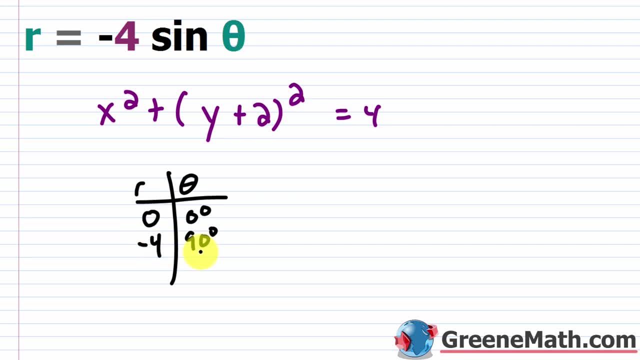 then r would be negative four. Now, if you want to convert that over, you could do positive four and 270 degrees if you wanted to. Okay, It's a little bit easier to work with. Now let's think about some other things. Where is sine equal to a half? Because if this was a half and I multiplied 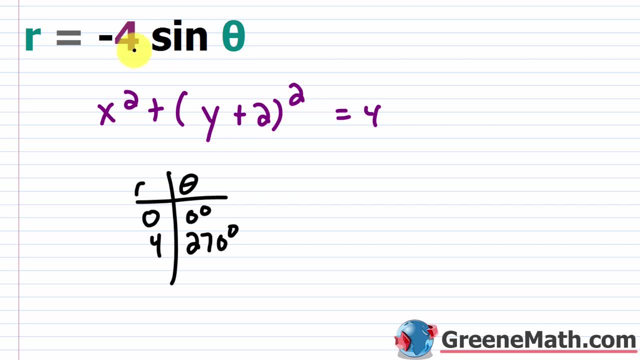 it by negative four better. yet if it was negative a half and I multiplied it by negative four, I would get positive two, Okay. So sine is one half at 30 degrees or 150 degrees. If you want it to be negative one half, then you would want to do 210 degrees. Okay, That would have a 30 degree. 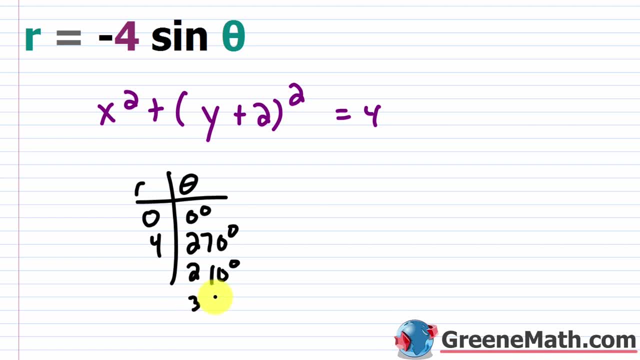 reference angle, Or you would also want to do 330 degrees, That would have a 30 degree reference angle as well. So in each case, sine of those sine of 210 degrees that would have a 30 degree reference angle, Or sine of 330 degrees, would be negative, one half, Negative four times negative, one half. 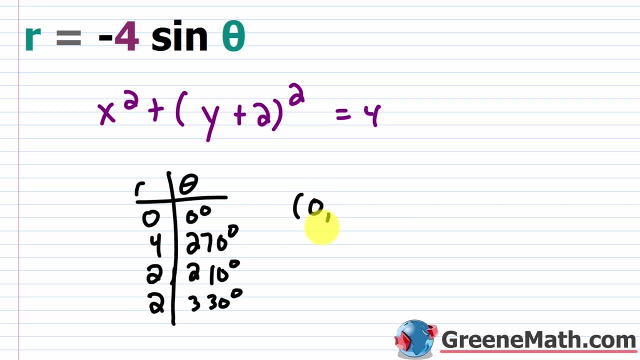 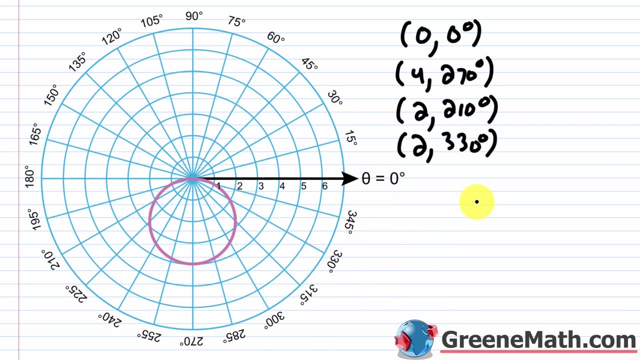 would give you two in each case. Okay, So let's write these out: We have zero comma zero degrees, We have four comma 270 degrees, We have two comma 210 degrees And we have two comma 330 degrees. Okay So, let's grab these guys. So zero comma zero degrees, that's obviously at the pole. So let's. 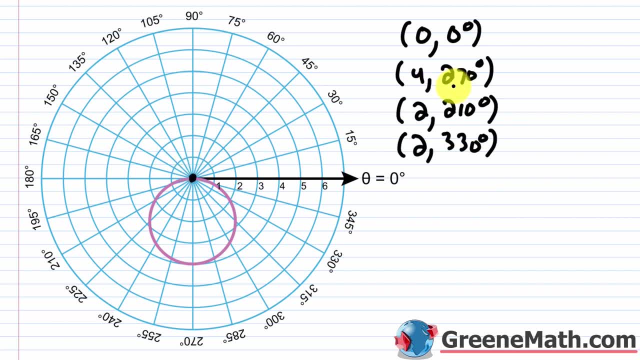 go ahead and highlight that. Then four comma 270 degrees go out to a circle with a radius of four. We're going to swing around. okay, to 270 degrees. So that's going to be right there. We have two comma 210 degrees, So let's go out to a circle with a radius of two. We're going to swing around. 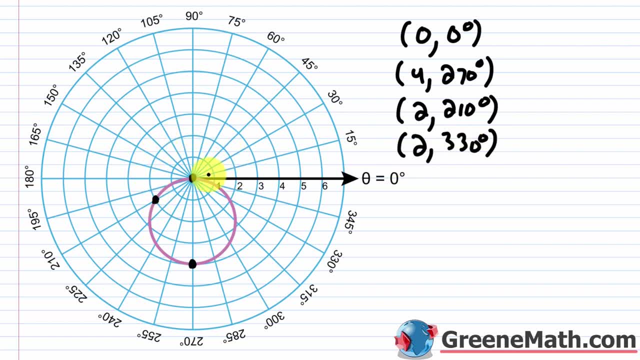 to 210 degrees. So it's going to be right there, And then two comma 330 degrees go out to a circle with a radius of two, And then we're going to swing around to 330 degrees, which is going to be. 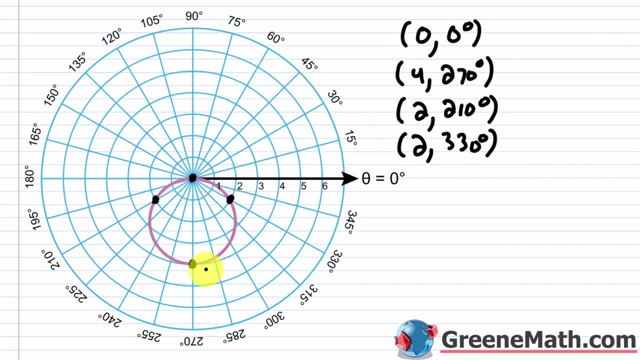 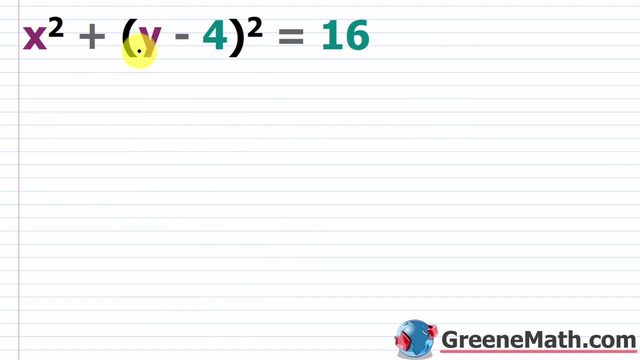 right there, Okay. So again, if I have four points, that's enough for me to come through here and sketch that guy as a circle, Okay? So look at another example. So we have x squared plus the quantity y minus four, squared equals 16.. Again, you're going to use 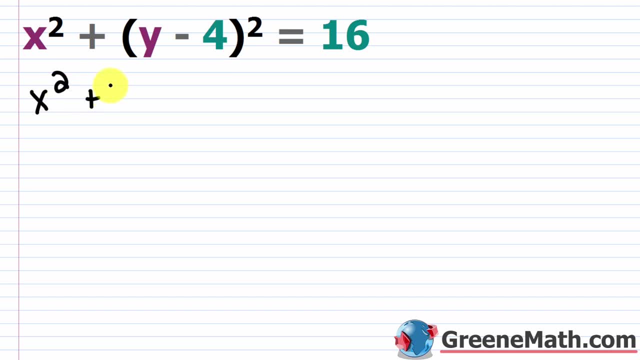 this formula, make sure it matches up. So x squared plus, you have y minus. a being squared is equal to a squared. So you've got to look at this guy and this guy, right? So is this guy being squared? giving you this guy, In this case, a is four, right, Not negative four you're taking. 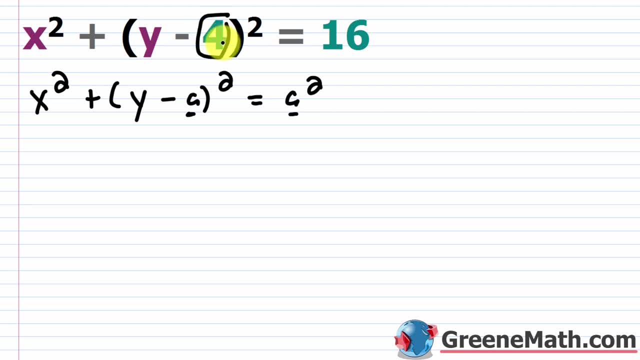 this right here: It's minus whatever this is, So a is four. If I square four, would I get 16?? Yes, If this was 17 or 18 or 19 or 20, that was not 16, then you could not use this formula because it does not work. Okay, So this: 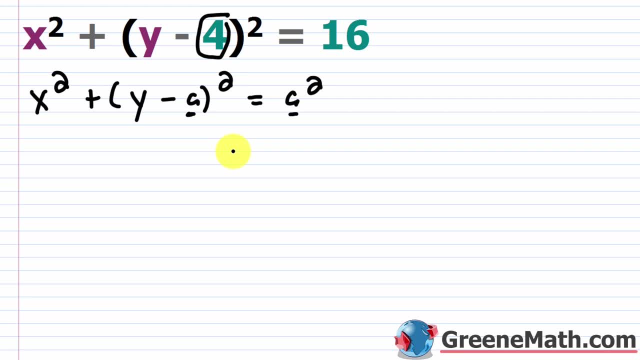 guy is going to give you the circle that passes through the origin and it's centered on the y axis. Again, this converts over to: r is equal to two multiplied by a times the sine of theta. Okay, So if I know a is four, then r is equal to two times four, which is eight times the sine of. 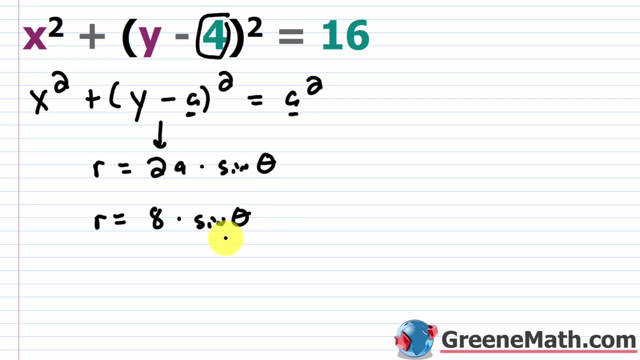 theta. Okay, So if you know the formula- and you get these a lot, these are very common problems- You can convert them almost right away. Okay, So let me erase this And again, I'll show you how to do this the long way. So what I would do. 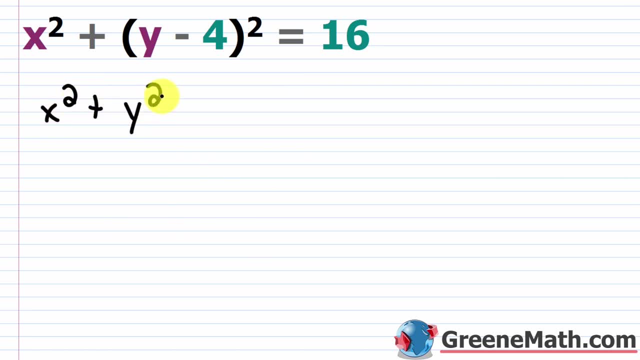 is: expand this So I'd say x squared plus y squared, And then you'd have minus two times this guy times this guy. So two times four is eight, and then times y, and then plus four squared is 16, is equal to 16.. And you'll notice that again, this is going to cancel. So what you have, 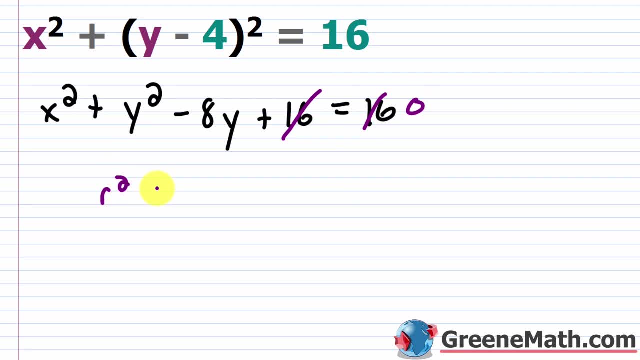 here is x squared plus y squared, which is r squared, And then I'm going to say is equal to. I'm going to add eight y to both sides, And then y. I can always replace with r, Okay. I can always replace with r- times the sine of theta, Okay. And again I can just divide both sides by r, You get. 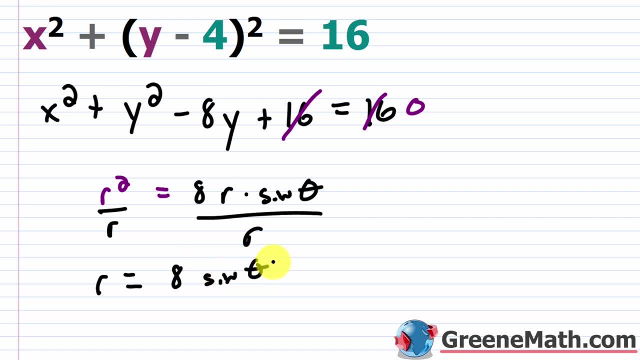 r is equal to eight times the sine of theta. Okay, So pretty quick to do that way as well, but the formula is actually faster, Okay, So let's go ahead and get rid of this And let me write this a little bit more neatly. So r equals eight times the sine of theta. Okay, So let me go ahead and 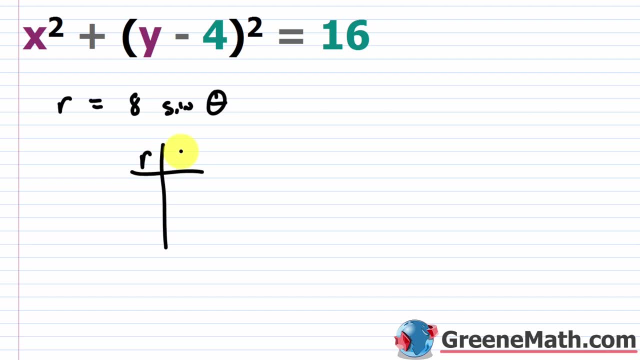 make that theta a little bit better. So let me go ahead and get some points for us. So r and then theta. Okay, So we know again, if I choose a zero here, so zero degrees, sine of zero degrees is zero. So this would be zero. Okay, If I choose 90 degrees, well, the sine of 90 degrees is one. So r. 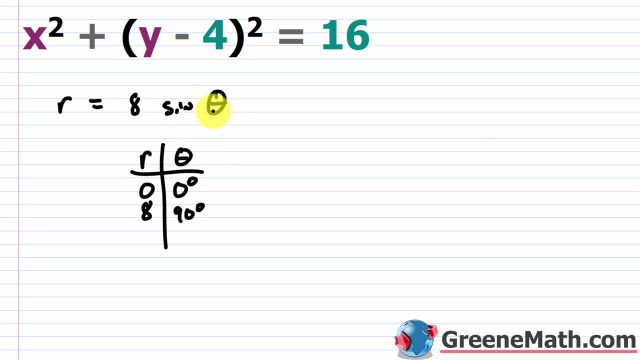 would be eight. Okay, And then I'm also going to deal with a half. Sine of 30 degrees is a half. So if I put 30 degrees here, that's a half A half times eight is four. And then, if I did, 150. 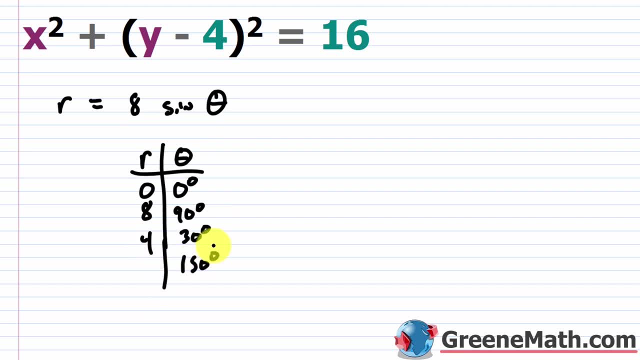 degrees. sine of 150 degrees is also a half. Eight times a half is four. Okay, So my points here would be four comma zero degrees and then eight comma 90 degrees, and then four comma 30 degrees and then four comma 150 degrees. So let me grab this real quick And let's go ahead and paste this in. 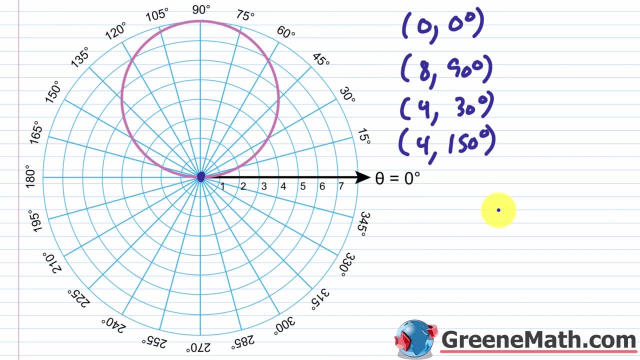 So zero comma zero degrees is going to be right there, If you want eight comma 90 degrees, so we're going to go out to a circle with a radius. We have one, two, three, four, five, six, seven. 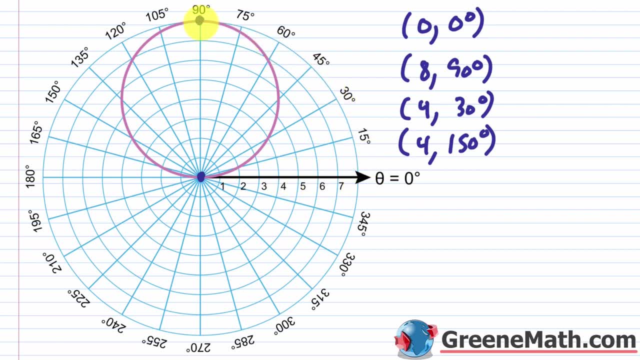 and then eight, And then I'm going to swing around to 90 degrees, So it's going to be right there. And then I want four comma 30 degrees. So I'm going to go out to a circle with a radius of degrees, So a circle with a radius of four, and then I'm going to go to this angle here of 30. 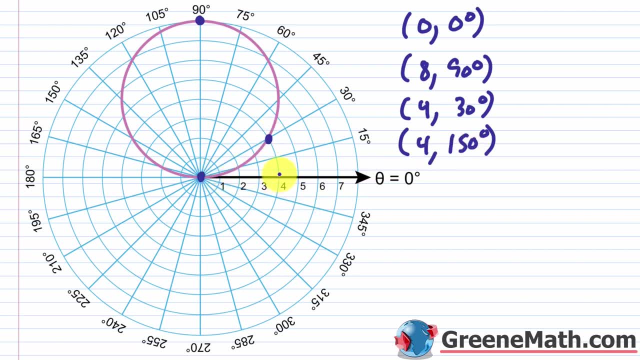 degrees and then four comma 150 degrees go out to a circle with a radius of four. I'm going to swing around to 150 degrees, So right there, Okay. So again, four points is usually enough. If you need more, you can approximate some of these other ones that are not going to be whole numbers in. 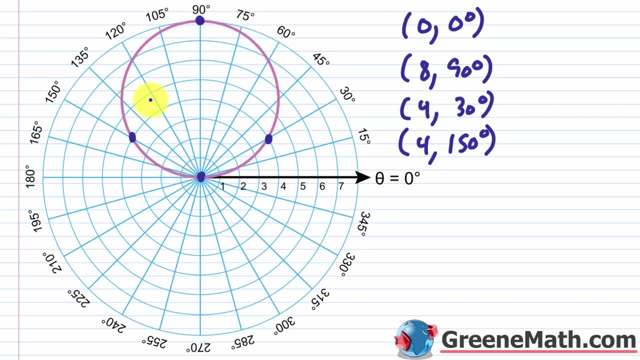 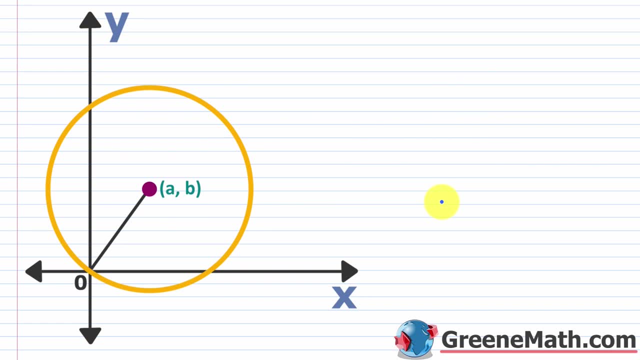 terms of the R values, but you can get very close to where you can sketch an accurate graph, All right. So let's wrap up the lesson and look at some examples where we're not centered on the X-axis, We're not centered on the Y-axis, We're not centered on the Y-axis, We're not centered on 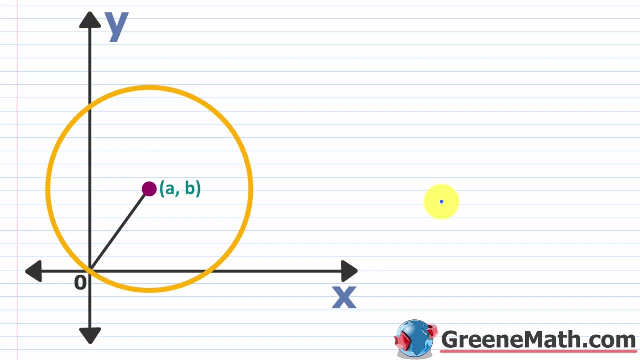 the Y-axis, but we're still going to have our circle pass through the origin. So, to set this up, I'm going to be working with rectangular coordinates, And so let me write this out: We have X minus H, quantity squared plus. we have Y minus K, quantity squared equals R squared. 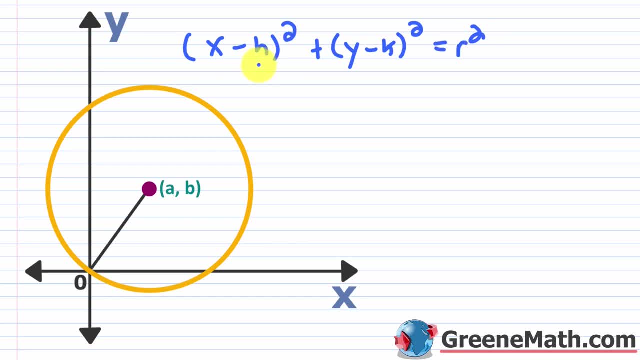 So this is back to basic algebra. I'm going to be replacing things. We can see that this passes through the origin- okay, which is the point in rectangular- as zero comma zero. We can see that the center, okay, right here is labeled with rectangular coordinates. 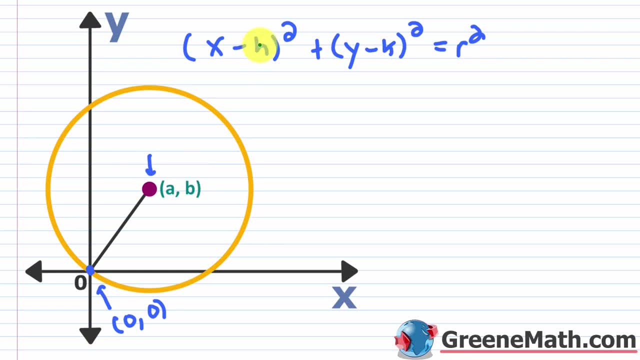 A comma B. So the X location is going to be A, So I can erase this and put an A, And the Y location is going to be a B, So I can erase this and put a B. Okay, Now again, you've seen me throughout. 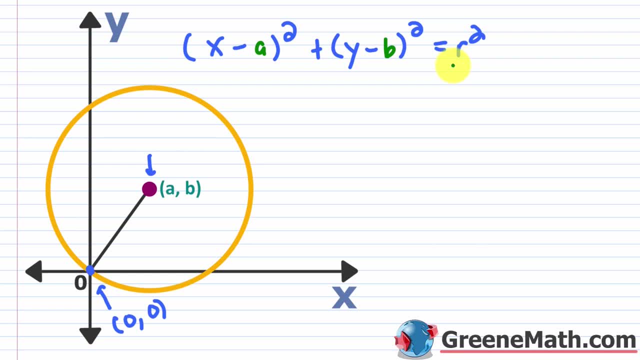 the lesson, replace this typical R that we see in algebra for the radius with A, because we don't want to get confused with the R that comes up in polar form. So for right now, I'm just going to erase this all together And I'm just going to put a blank here in square. Okay, So what would I? 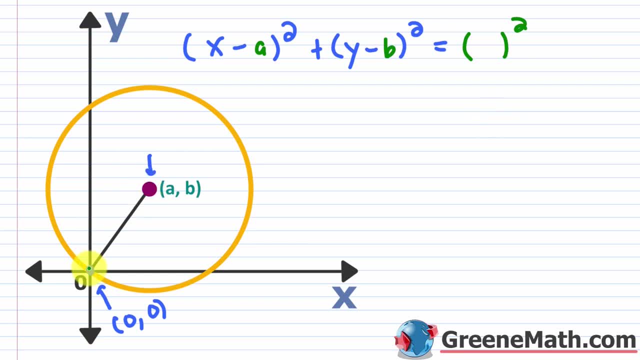 need Remember. the radius is the distance from the center to the center. So I'm going to put a blank here in the center to any point in that circle. So the distance from right here to right here can be found with the distance formula, if you want to use that, So you could say the distance. 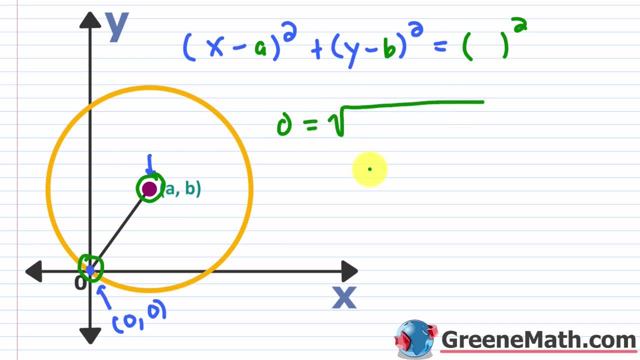 between these two points would be the square root of what. Well, you would subtract A minus zero, right? You subtract the X coordinates, So let's say A minus zero would just be A, and you're going to square that. Then, plus, you're going to subtract the Y coordinates, So B minus zero would. 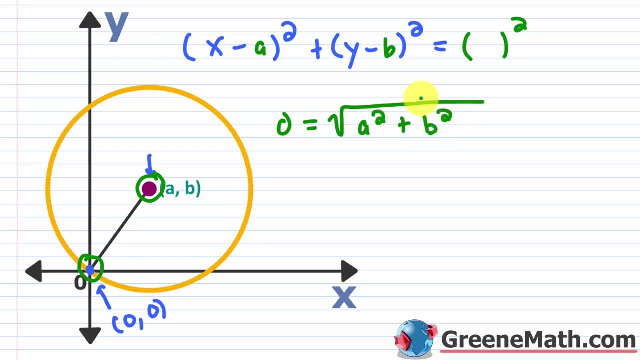 just be B and that would be square. Okay. Now if I put this in here and squared it, I would just get A squared plus B squared. So let me erase this and just put A squared plus B squared, Okay, So that's really all there is to this formula when you see it in rectangular. 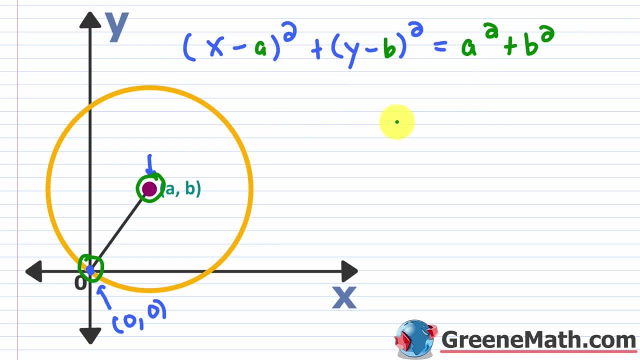 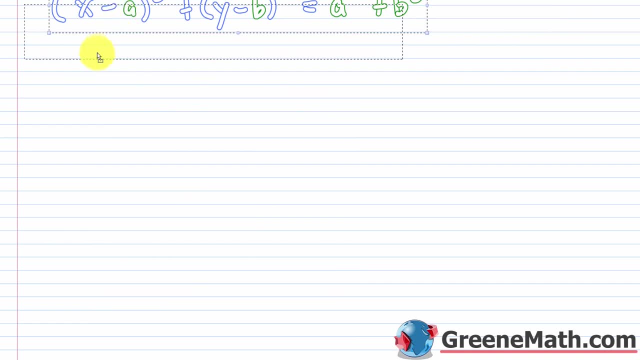 form. When you convert it over into polar form, it actually works out quite nicely. So let's grab this guy real quick, Let's copy it and let's paste it on this fresh sheet here. Let's see what we can do. All right, So from here, what I'm going to do is put this into polar form. We're going to find 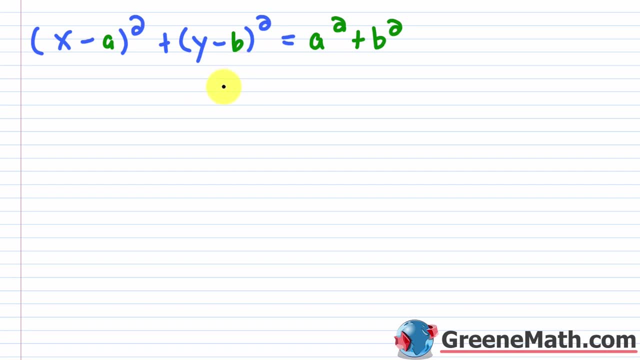 this is really, really useful when we're trying to convert back and forth between the two. So I'm going to start by expanding this guy and this guy on the left-hand side, So we already know how to do this. This is X squared minus two times this guy times this guy. So minus two AX. 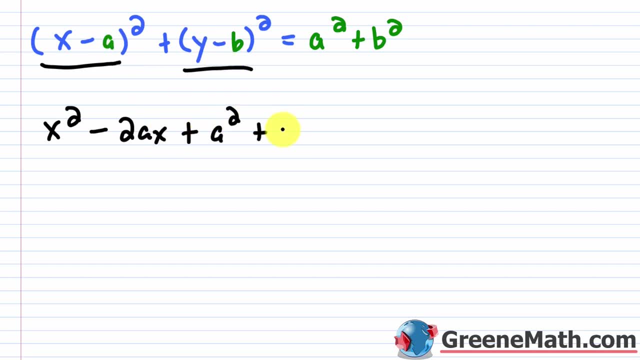 then plus this guy squared, So A squared. then plus same thing over here, So Y squared, minus two times this guy times this guy, So minus two times B Y. then plus this last guy, B squared, And this equals A squared plus B squared. Okay. 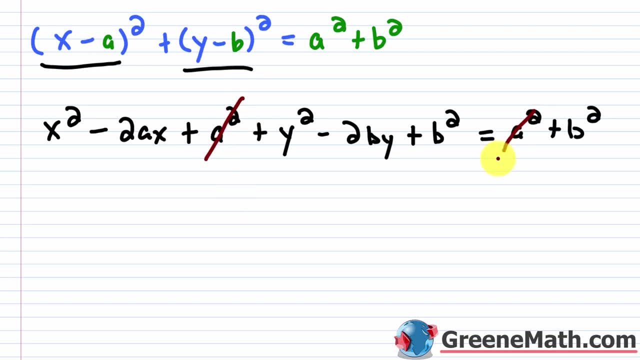 So we can see that this is on each side, right? So I can subtract away from each side and it's going to go away from each side. This is on each side, So I can subtract away from each side. It's going to go away from each side because everything is gone on the right-hand side. I'm going to put. 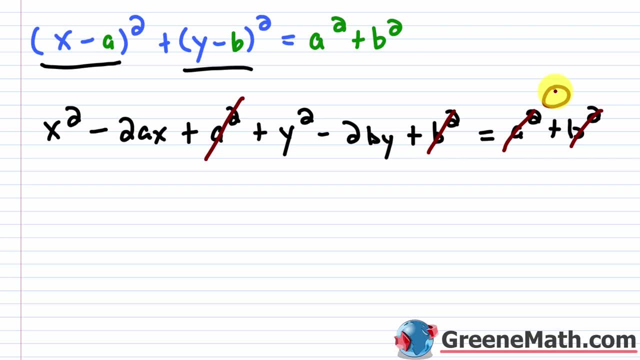 a zero there. Okay, So over here, what I can do now is rearrange things. So I'm going to put the X squared plus the Y squared next to each other. Again, that's a common theme. where you're working with these problems, You're trying to get the polar, So I'm going to say X squared plus Y. 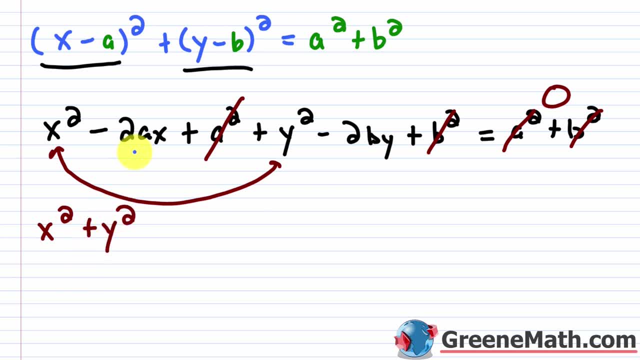 squared Again. you can replace that with R squared. Then what I'm going to do is I'm going to take this guy and move it over here, And I'm going to move this guy over here as well. So let me put my equals here. I'm going to add: 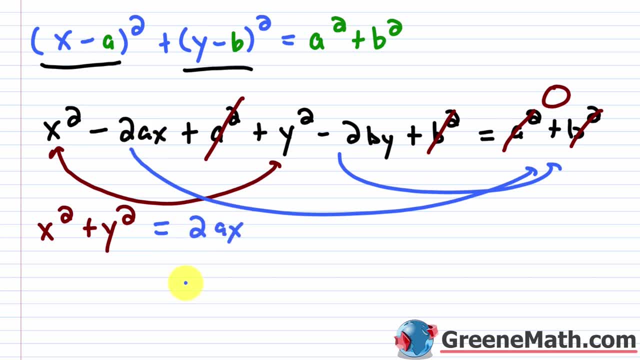 two A- X to both sides, So of course it's going to cancel over here. And then I'm going to add two B- Y to both sides, So again, of course it's going to cancel over here. Okay, So this is my. 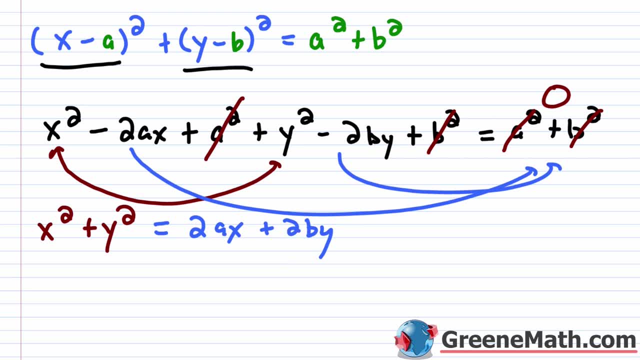 equation now And basically to convert it over to polar: X squared plus Y squared is R squared by definition. And then everywhere I see an X, I can always put R cosine theta. So I'll put two A times R cosine of theta, and then plus two B. everywhere I see a Y, I can put R and then sine. 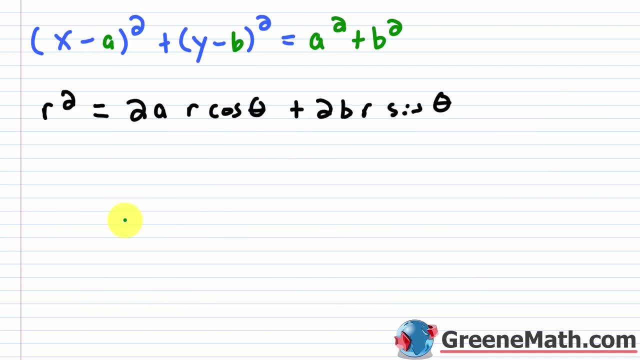 of theta. Okay, Let me erase all this. And essentially, what you want to do here is solve this for R. Again, the common mistake is to take the square root of each side. What you want to actually do is factor this R out, Okay. So factor this R out so that you can divide both sides by. 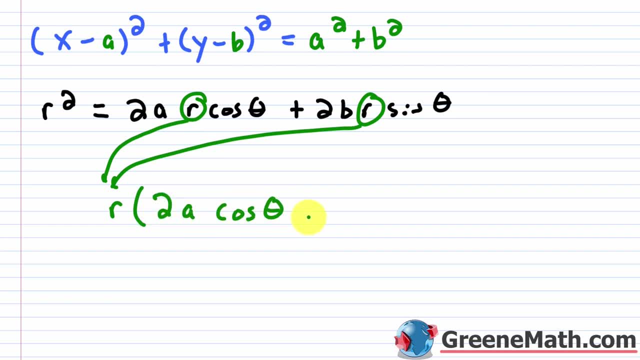 R. So I'll say this is two A times the cosine of theta, and then plus two B times the sine of theta. Okay, So that's going to be equal to the R squared. Okay, So again, the trick here is: I'm going to 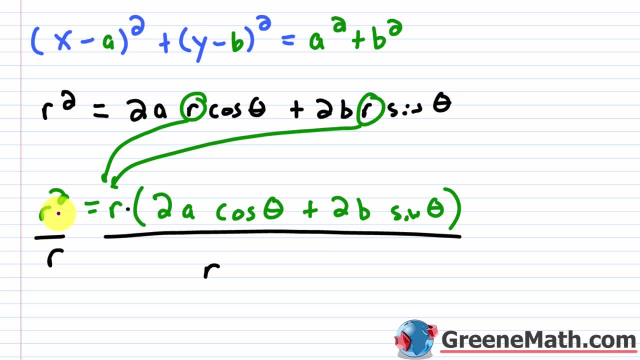 divide both sides by R. This is just multiplication here, So this is perfectly legal. Cancel one of these with this. cancel this with this, Okay. And what I'm left with? let me just write this above here, Okay, Cause we're going to use this. We'll say in polar form: this is: R is equal to. 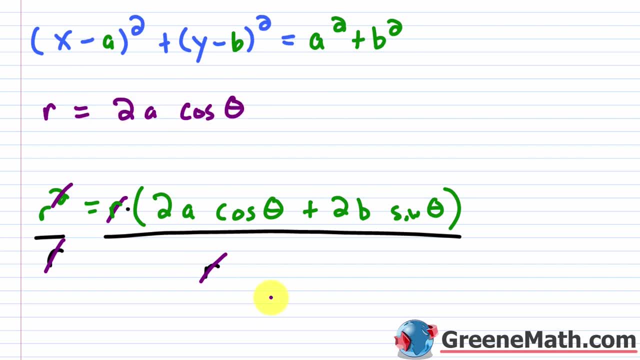 you'll have your two A times the cosine of theta, Okay, And then plus your two B times your sine of theta. So there will be a lot of problems that deal with this calculus and in calculus Again, this is for a very specific case- Your circle is going through. 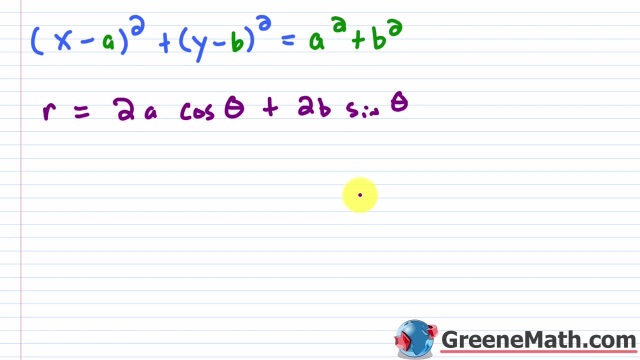 the origin. Okay, And then your center is not on the X axis, It's not on the Y axis, The center, let me write this again. So the center is going to be at A comma B. Okay, And then you want to check. 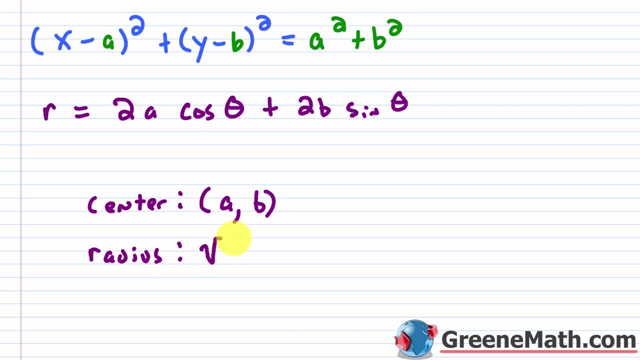 that your radius. your radius again is the square root of A squared plus B squared, Okay. So if your circle fits this description okay in rectangular, then you can quickly convert it over to polar using the R. So that's going to be A comma B, Okay, And then you want to check that your radius. 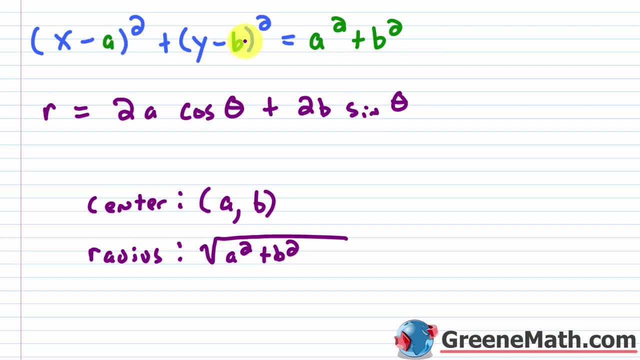 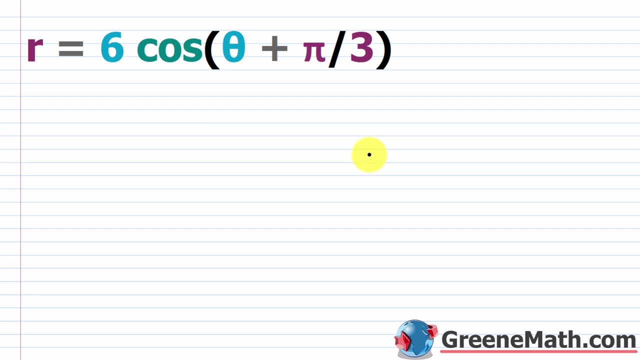 this form here. Okay, So you take your A from here and your B from here. You can check that A squared plus B squared is what you've got here. is your number, Okay, And then you can convert it over. All right, Let's take a look at an example. So we have: R is equal to six times the cosine of. 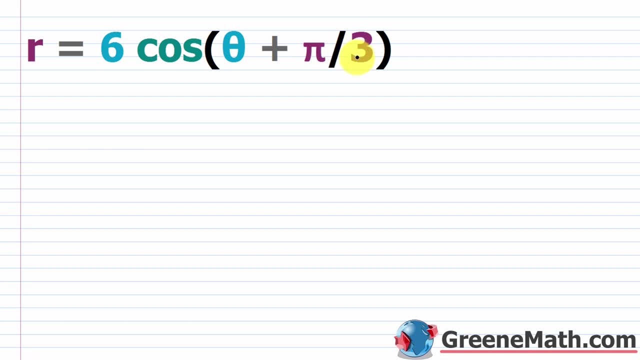 we have this theta plus pi over three. Okay, So the first thing I would do here is just simplify this using my cosine sum identity. Okay, So I'm going to say R is equal to. I'm going to put six. You can use parentheses or brackets, whatever you want. 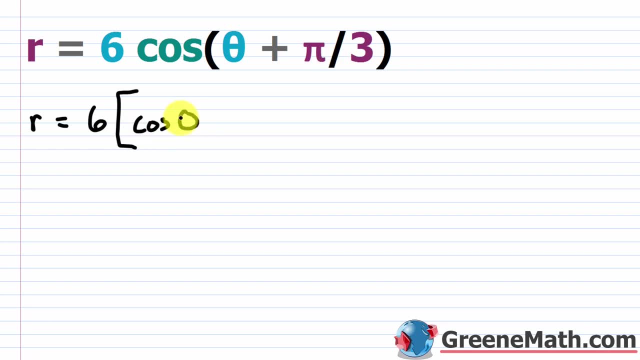 expand this out. So I'm going to say: this is the cosine of theta and then times the cosine of pi over three, And then remember, when you use the cosine sum identity, your signs are going to change. This is plus, so it's going to be minus, So this is now going to be the sine of this theta. 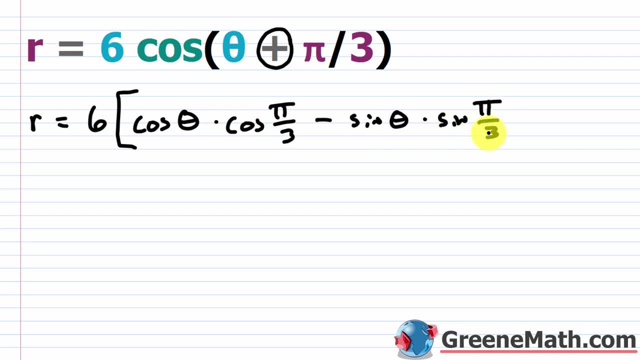 and then times the sine of pi over three. Okay, Close these brackets down. We know pi over three is 60 degrees and cosine of 60 degrees is a half. We know sine of pi over three or sine of 60 degrees is square root of three over two. So let's just replace that real quick. I'll say: R is equal. 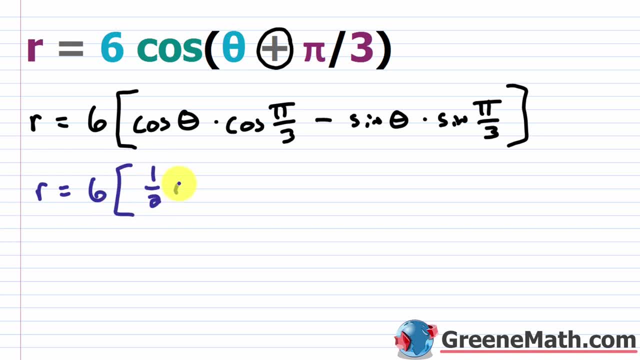 to six. open up the brackets. I'll say one half times the cosine of theta, and then minus, I'll say square root of three over two times the sine of theta. Okay, Now when you distribute the six into each, you have a denominator of two. six divided by two is three, So you basically have three times. 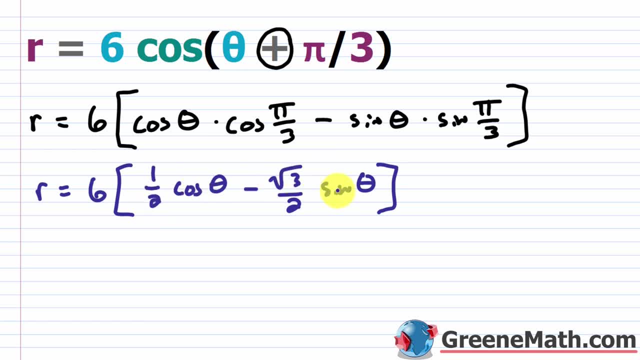 cosine of theta and then you'd have negative three times square root of three times sine of theta. Okay, So let's go ahead and say we have, R is equal to, again, this would be three times cosine of theta and then minus three times square root of three times the sine of theta. 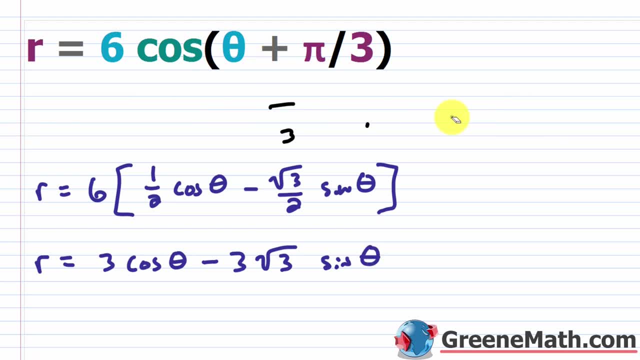 Okay, So here's where we can stop. I'm just going to erase all of this. We don't need it anymore. All right, So to use the formula, let's just write: R equals our two A times the cosine of theta. 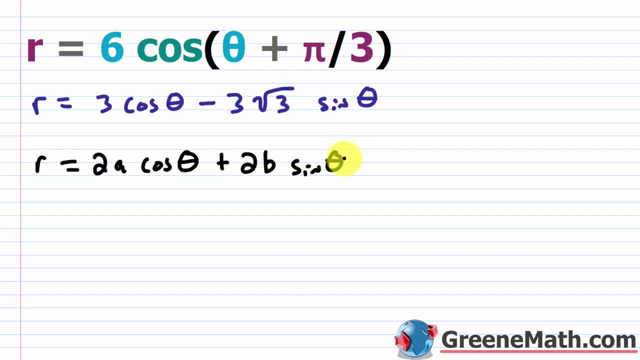 then plus the two B times the sine of theta, This converts over to X minus A quantity squared plus Y minus B quantity squared is equal to A squared plus B squared. Okay, So if I'm trying to convert this over here, I know that two A. I just got to match these things. 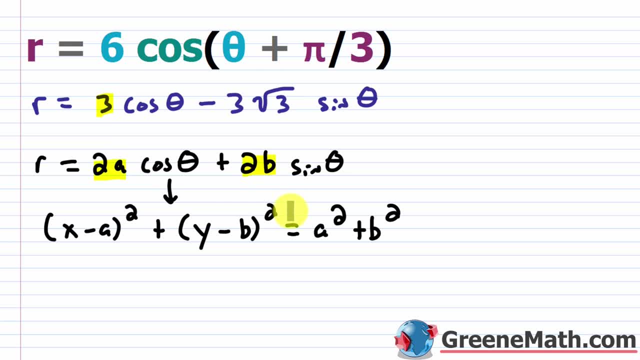 up: Two A is equal to three and two B- Okay- Is going to be equal to the negative of three times square root of three. Okay, So be very, very careful there because, depending on your book, you might get different formulas. So I'm going to say that two A is equal to three. 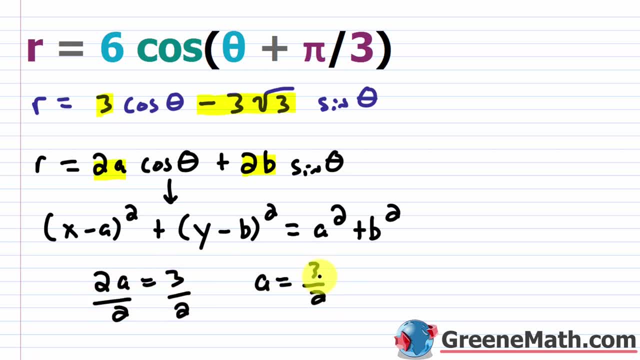 divide both sides by two and A is equal to three halves. Okay, So that would get plugged in here and here. Okay, So let me erase this And actually put this up here. So A is equal to three halves And then, similarly, if I have two, B is equal to. 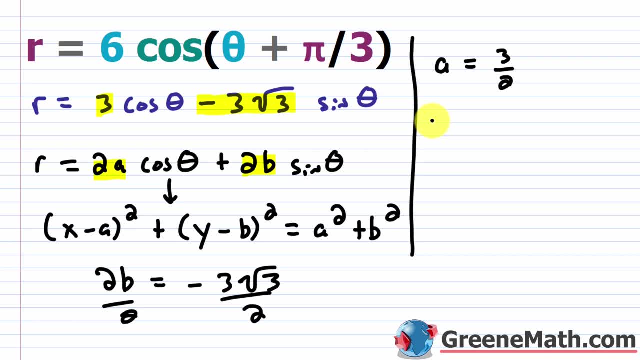 negative three times square root of three. we'll divide both sides by two, and B would be equal to the negative of three times square root of three over two. Okay, Then make this three a little bit better, Okay, And then again you're just plugging in. So if I took that and I plugged in here, 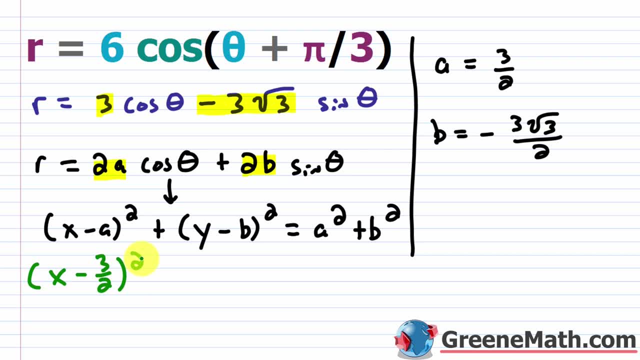 so X minus three halves. this quantity would be squared and make these parentheses a little bit larger. Then plus You would go. Y minus. a negative is plus positive, So Y plus. I'll go ahead and say three times square root of three over two. quantity squared is equal to: So you've got a square A, you've got a. 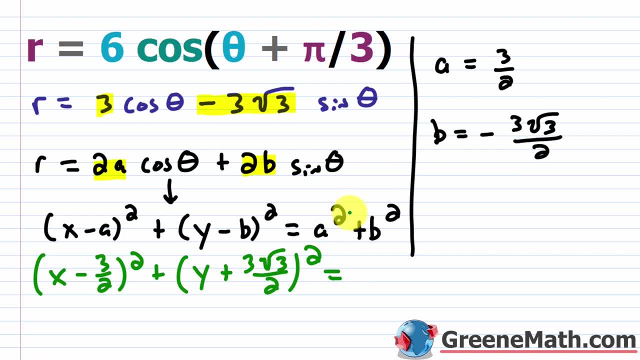 square B, and then you want to sum those results. So A squared three halves squared, is going to be nine fourths. Then, plus if you square this guy, the negative becomes positive. Three squared is nine. square root of three squared is three and two squared is four. So basically this is 27 fourths. 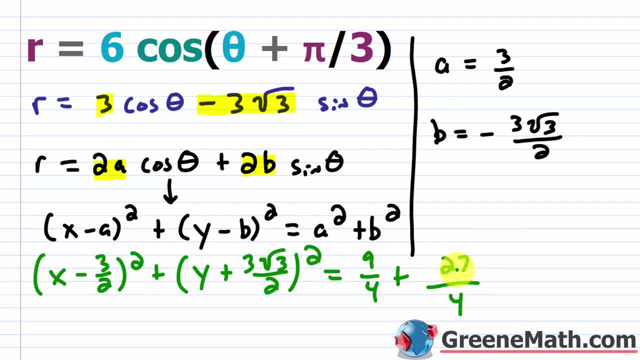 If you add these guys together, because you do have a common denominator, you're going to get 36 over four, which is nine. Okay, So this right here would be how you can quickly convert- And I say quickly, but how you can more quickly convert this over to your rectangular form, I realize. 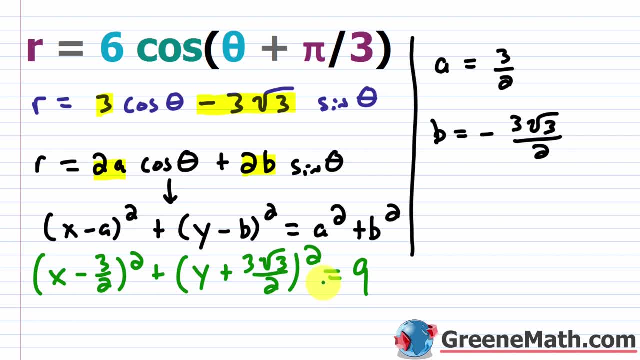 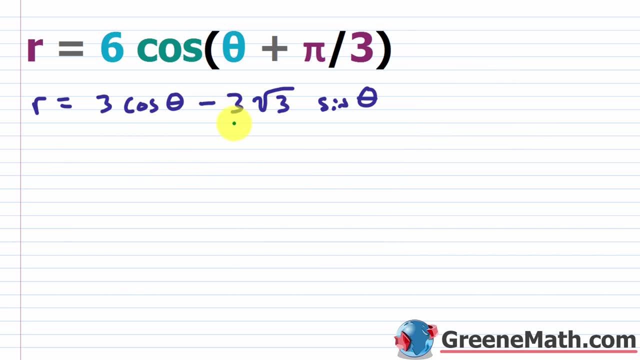 this problem does take some time, no matter how you do it, Okay. So what I would do from here, let me just erase this and I'm just going to do this the long way, Okay? So when you see something like this, you think I'm going to be doing a couple things at a. let's just call it a linear. 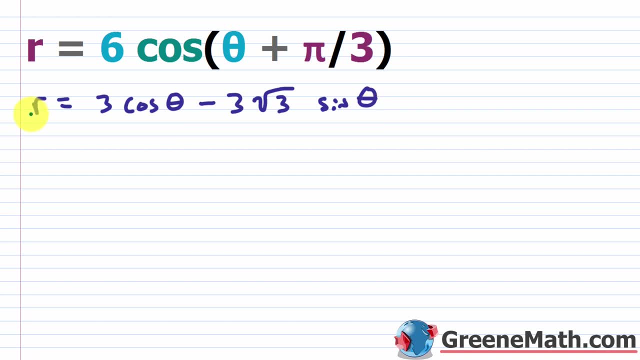 formula. Well, what you would want to do is you would want to remember, and you remember that we always Do not argue that point and we just have to break it down to these two real things to do is multiply both sides by r, or the way you do it. So if I do this, we'll take the choose plus time, and 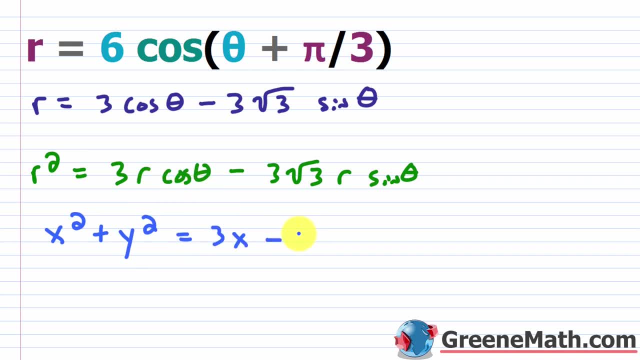 we're going to come up with the term of gamma as well for intelligence and equation, And I again really minus. this is going to be three times square root of three and then times y. Now, if you feel more comfortable, you can write the y right here, so you could also write this as negative: three times y. 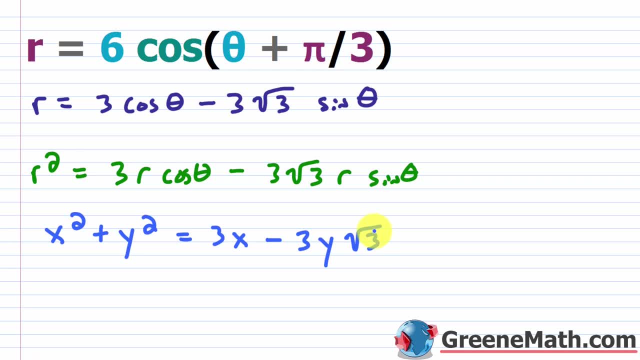 times square root of three. A lot of books will do this so that you don't get confused and think that the y is underneath the radical there. so we'll just kind of use this notation. but the coefficient for y is negative three times square root of three. so we have to know that, Okay so, 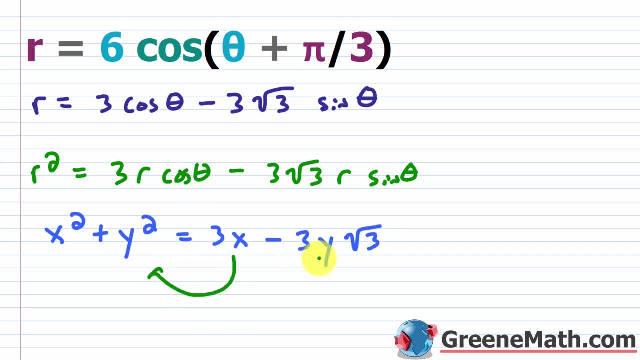 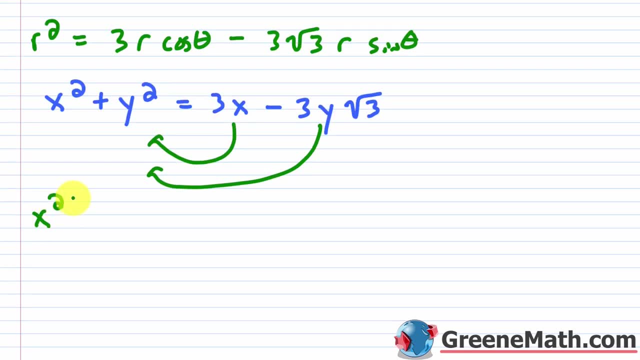 what I want to do now is move things over. so I want to move these guys over here, okay, and the reason I'm going to do that is so that I can complete the square. So if I subtract 3x away from both sides, I'm going to have x squared, I'm going to have minus 3x, then I'm going to put plus. 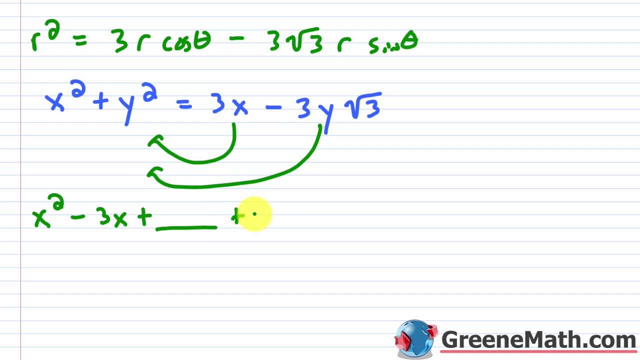 and I'm going to leave a space right because I want to complete the square. Then plus I'm going to have my y squared. I'm going to add this to both sides. so plus 3y times square root of three. okay, then plus I'm going to leave space, and this equals I'm going to put zero. So what I would do. 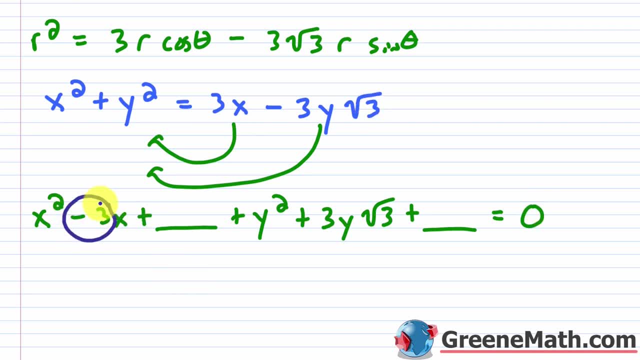 here is complete. my square again. take the coefficient for your variable raised to the first power. So in this case it's negative three times square root of three. So I'm going to add this to the first power, So I'm going to cut it in half. so that would be negative three halves Square it, you would get nine fourths Okay. 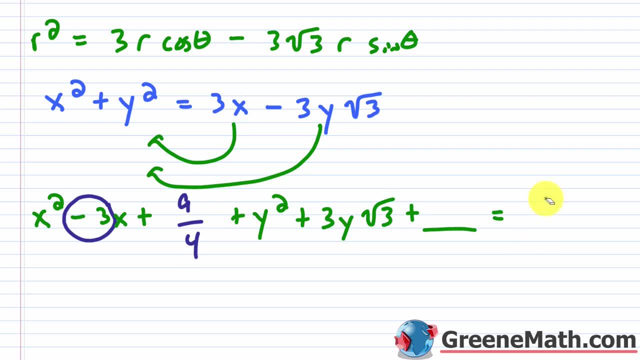 so let me write nine fourths here. Again, it's not legal to do this unless you add it to both sides, So we got to put it over there. Okay, then over here. this one is a little bit more tricky, but we just did it. It's three times square root of three. Cut it in half and I'm writing these: 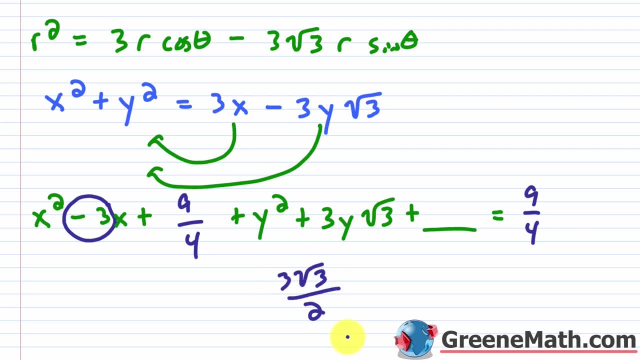 threes, terribly. So let me put this in a little bit better form here. Cut it in half and then square it. We just saw this is going to be 27 fourths. So this is 27 over four. Okay, so plus 27 fourths- We already know this becomes 36 fourths, and this is not right, because we basically 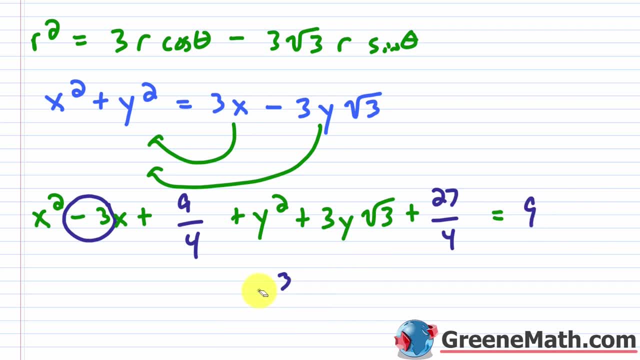 just did this, So this is nine. Okay, and again, if you go through and factor these, this is a perfect square trinomial, and this is a perfect square trinomial. So this factors into x minus your three halves quantity squared, and then, plus this, is going to factor into y, plus your three times. 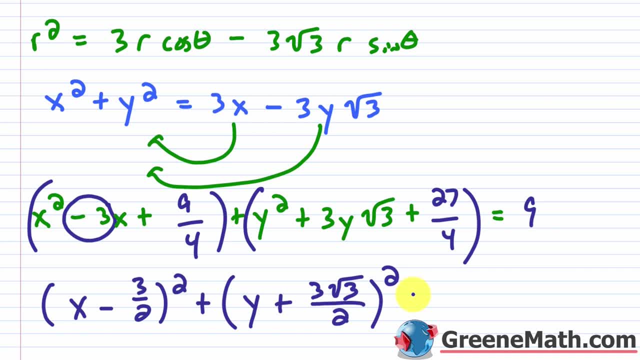 your square root of three over two, quantity squared, and this equals nine. So however you do this, you're going to get the same result. So I'm going to cut it in half and I'm going to put it over here. I just want to give you multiple ways to attack the same problem. Okay, let's erase all this In. 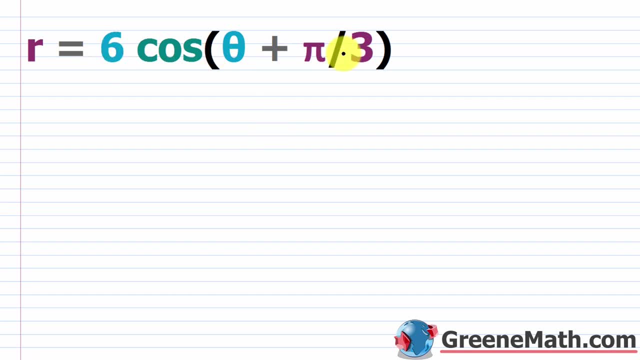 order to graph this on the polar grid. I'm going to use this form. It's a little bit easier when you just have cosine involved, versus having cosine and sine, because I can just plug stuff in here, then add the 60 degrees to it and then I can take the cosine of that, you know, so on and so forth. 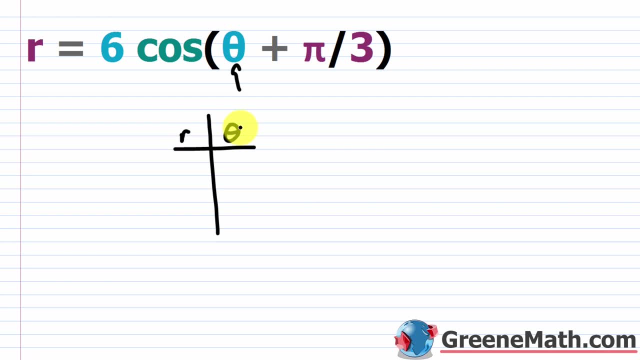 So I'll say r and then theta. here I've got to think about the fact that whatever I plug in there, I'm adding 60 degrees to it. So if I put in zero degrees, I add 60 degrees to that, I get 60 degrees. Cosine of 60 degrees is a half A half times six is three. 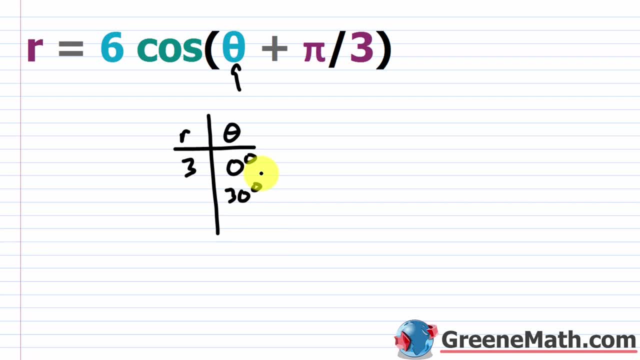 Then if I did something like, let's say, 30 degrees, Well, if I add that to 60 degrees, I have 90 degrees. Cosine of 90 degrees is zero. Zero times six is zero. Let's keep going with two more points. 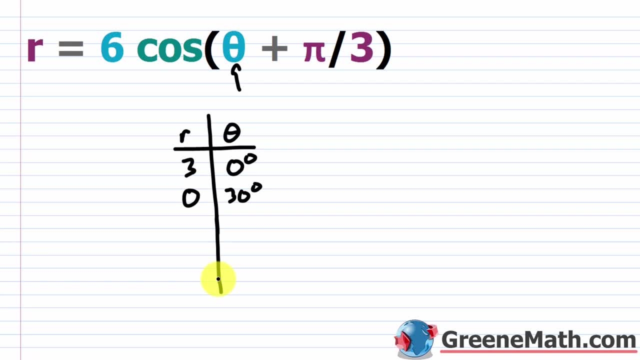 Again. I'm just trying to get some whole numbers here, So let me also do something like 240 degrees. 240 degrees plus 60 degrees would be 300 degrees. That has a 60 degree reference angle right and it's also in quadrant four, so it's going to be positive. So the cosine of 300 degrees is a half. 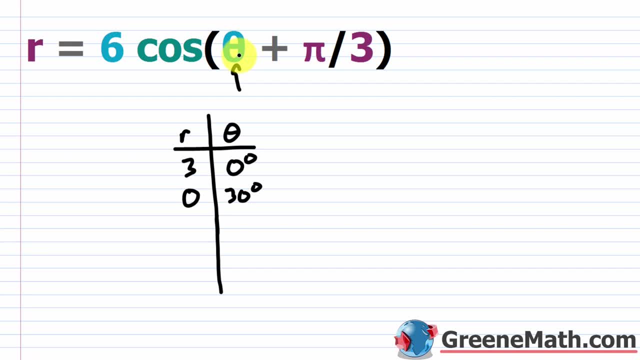 Six times a half, we already know is going to be three, right? So if this was 240 degrees, okay. again, adding 60 degrees gives me 300 degrees. Cosine of 300 degrees is a half. Six times a half is three, All right. the last thing I want to consider: we know that the cosine of zero degrees 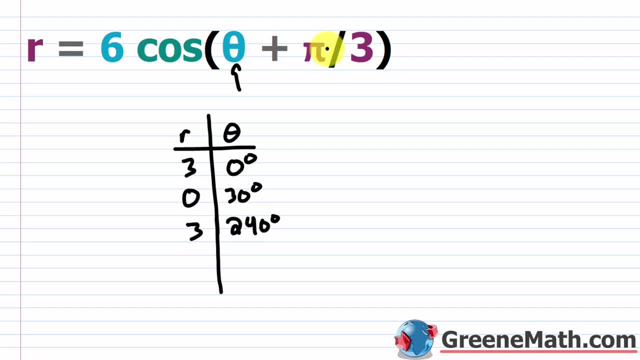 is one. okay, but again I'm adding 60 degrees to this. So let me go ahead and put 300 degrees in here. Okay, that's another one we can try. So 300 degrees plus 60 degrees, 360 degrees. Cosine of 360 degrees is the same as cosine of zero degrees. It's going to be one. 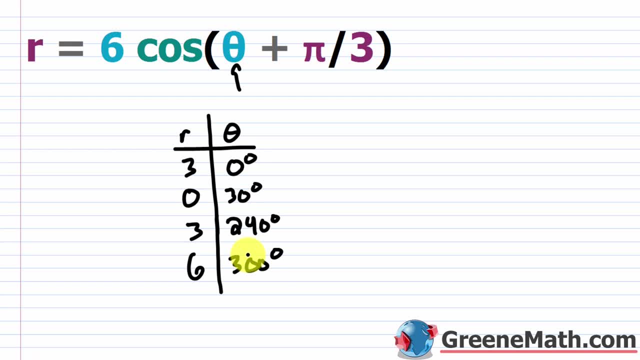 So six times one would just be six, Okay. so this is four points Again. if you need more, you can always use some approximations. I'm going to go ahead and say three comma zero degrees. I'm going to say zero comma 30 degrees. I'm going to say three comma 240 degrees, and then I'm going to say 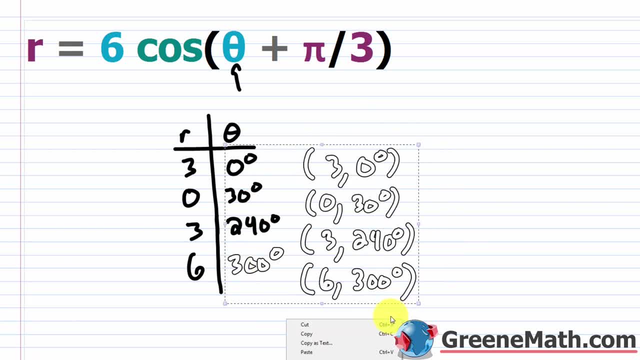 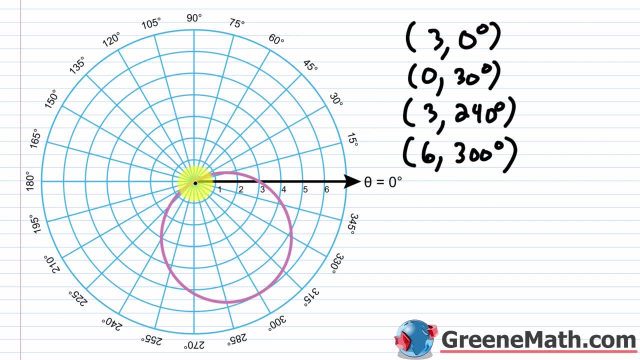 six comma 300 degrees, like this: I'm going to grab these guys, copy them. Let's paste this in here, like that, so we have it. So again, three comma zero degrees. Well, basically, from the pole, I'm just going to step out to a circle with a radius of three, So 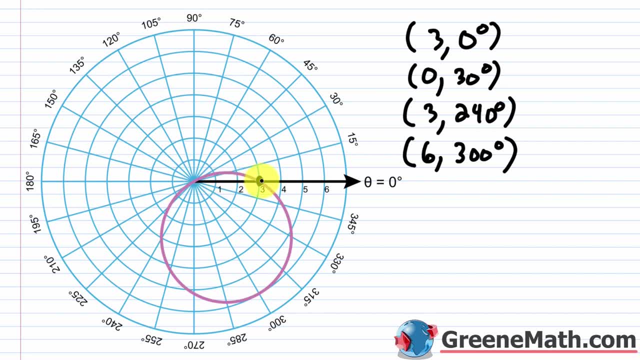 I'm just going straight to the right, like that. and then zero comma 30 degrees Again. if this is zero here for the radius, I'm not going anywhere right? So I'm going to be right there on the pole. Three comma 240 degrees. I'm going to step out to a circle with a radius of three Swing around here. 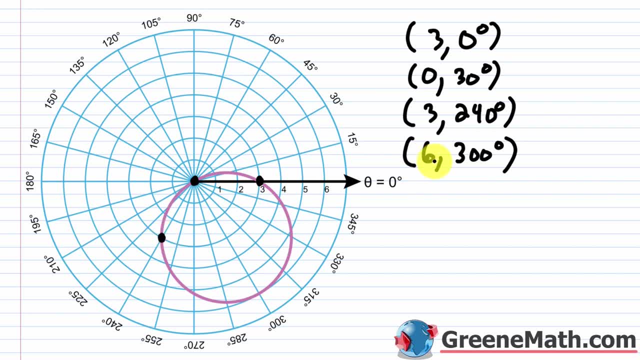 to 240 degrees. So it's going to be right there. Then you have six comma 300 degrees. So I'm going to go out to a circle with a radius of six. I'm going to swing around to an angle of 300 degrees. 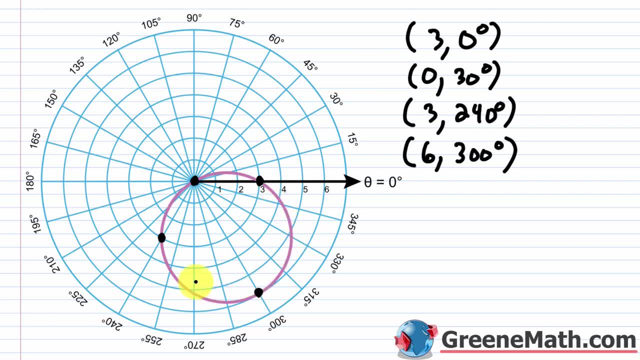 Let's go right there. So again, if you need some points in between these to make a more accurate sketch, you can use some approximations. Okay, that's up to you. Generally speaking, if you do this for a homework assignment and you show four points and you draw your circle through those, 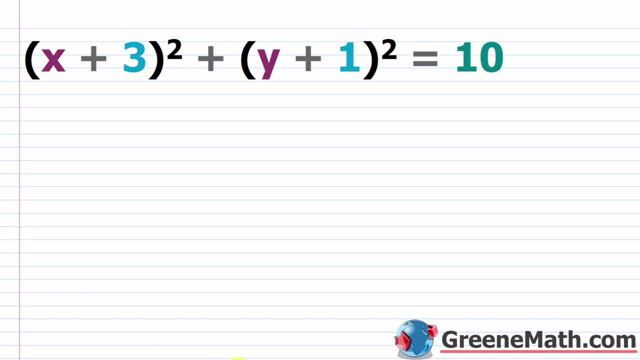 points, you're pretty much good to go, All right. so the last example here that we're going to do: we have x plus three quantity squared plus we have y plus one. quantity squared equals 10.. So for this again, I'm going to write this in the form of x minus a quantity squared plus we have y minus b. 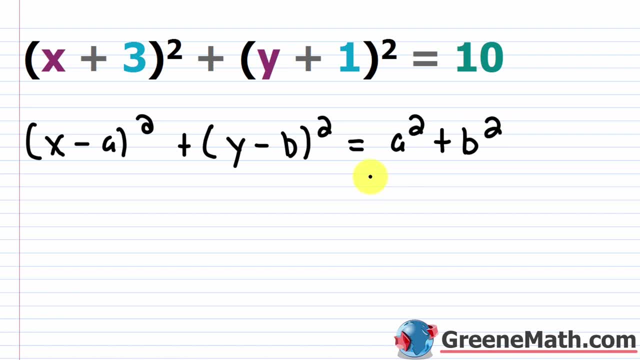 squared is equal to a squared plus b squared. So you first want to check to see if this matches up. So if you have plus some number, you have it here, and then here right is minus a negative. So I'll say x minus a negative three and then quantity squared plus, you'll have y minus a negative one. 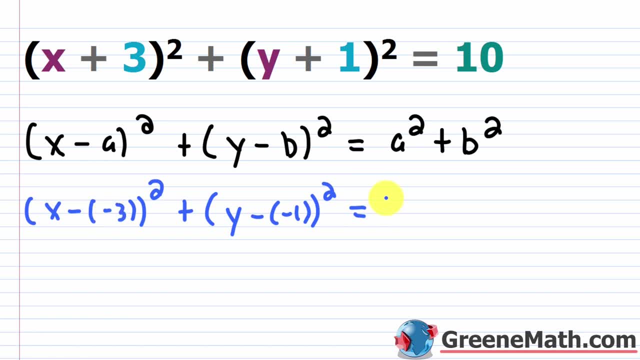 quantity squared is equal to. In this case, you'd have negative three being squared, So negative three being squared plus, you'd have negative one being squared. So first you want to check to make sure that this works out. If this was, let's say, 11, you could not use this formula. You could. 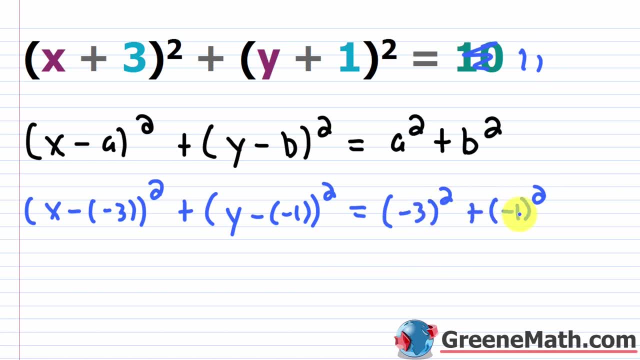 use this formula because it doesn't work out. Negative three squared is nine. Negative one squared is one. Nine plus one is 10, not 11, right? Or if it was 12 or 14 or anything other than 10, this is not going to work out, But since it does follow this format, what I can do is just grab. 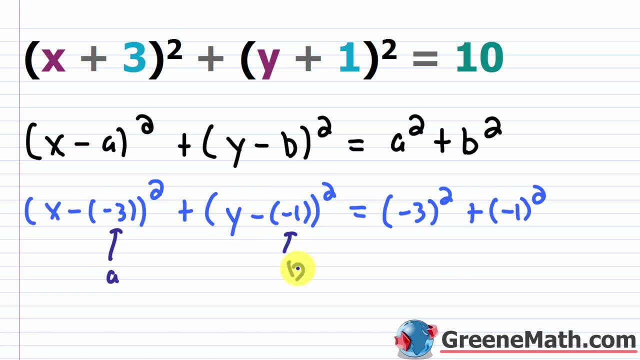 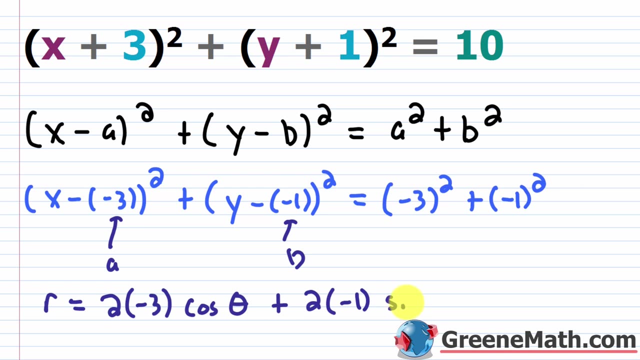 these values, So I can say this is a and I can say this is b, and then you can just plug in right, So you can say r is equal to well, I have two times a, so two times negative, three times the cosine of b. B is negative one times the sine of theta. Okay, and that's all you need to do. So let's come. 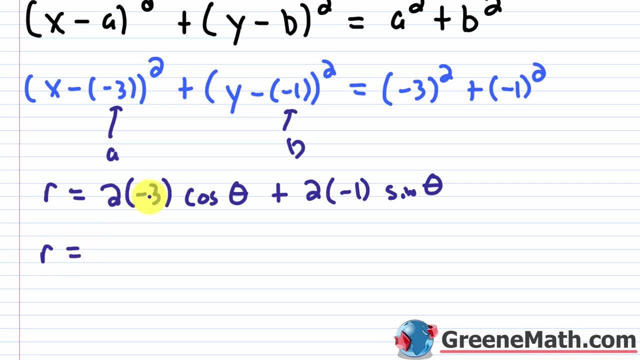 down a little bit. So this would be: r is equal to, we'll have two times negative three, which is negative six times the cosine of theta. Then we'll have two times negative one, which is negative two. So I'll just put minus two and then times the sine of theta. Okay, so this is converted into polar. 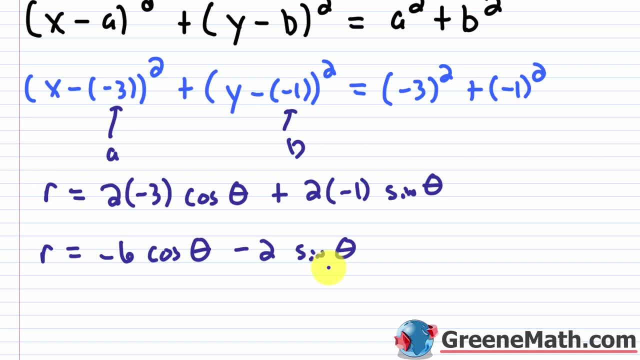 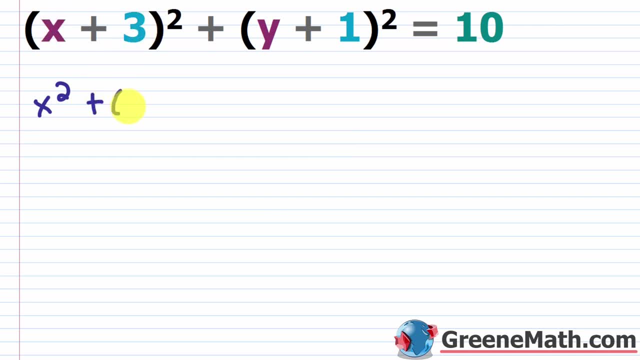 form Again, just for the sake of completeness, I'm going to do this one more time the long way, just so you get some practice. If I come back up here and I expand this, this is x squared plus two times this guy times this guy, So six x plus this guy squared, So nine plus this guy is y squared. 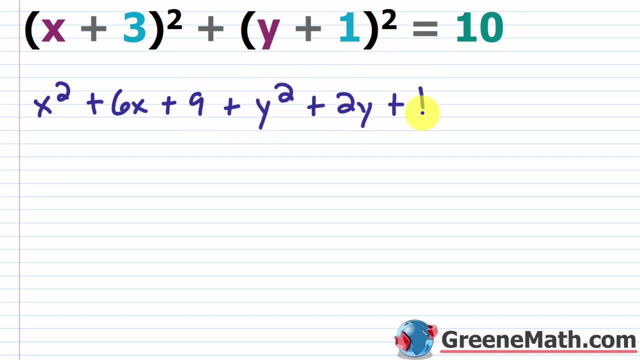 plus two times this guy times this guy, So two y plus this guy squared, which is one, and this equals ten. Okay, so if you sum nine and one, you get ten, and again you can subtract that away from each side. So I'm going to go ahead and line these out and line this out and put a zero right, Just like. 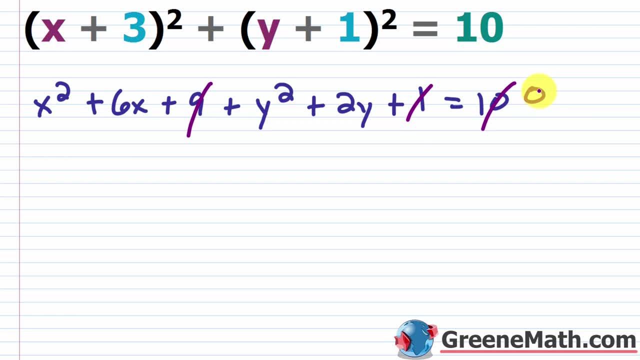 I subtracted ten away from each side. So then, from here, what I'm going to do is do my x squared plus y squared. I'll just go ahead and say that's r squared, and I'm going to say this equals. I'm going to move these guys over to the right hand side, So I'm going to subtract six x away from. 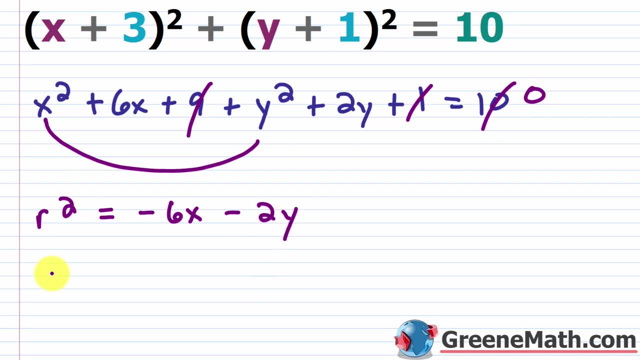 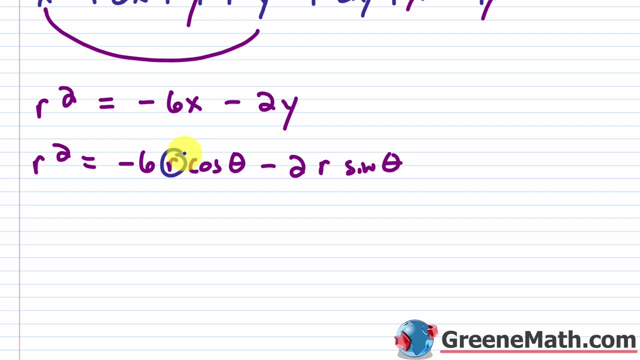 each side and I'm going to subtract two y away from each side. So then I'll have r. squared is equal to negative six times. this is r cosine of theta. then minus two times, this is r sine of theta. Okay, and then from there again you can always factor the r out. So you have it here and you. 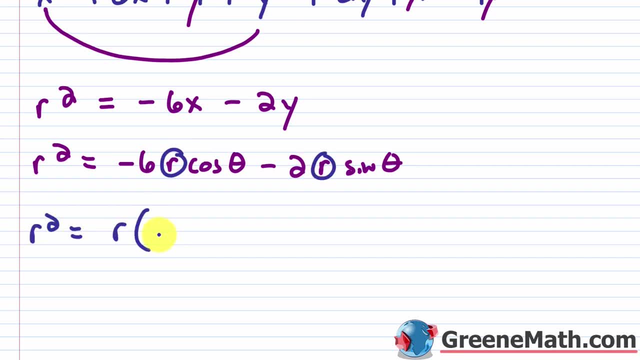 have it here. So let me write: r squared is equal to r times the quantity negative, six times the cosine of theta, then minus two times the sine of theta. Okay, and then let me divide both sides by r. So divide both sides by r and one of these will cancel with this. This will cancel with this. 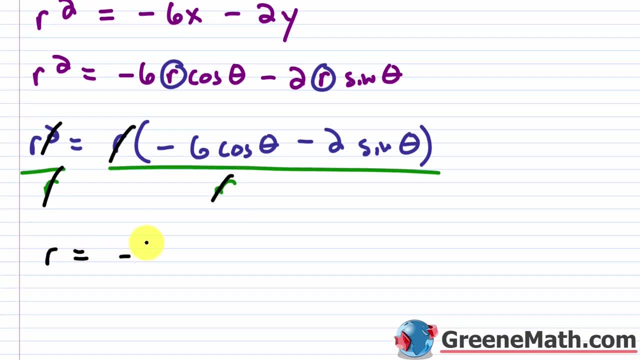 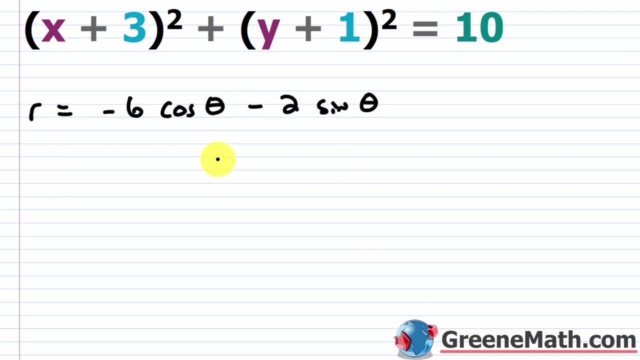 and you're back to that form that we found. So r is equal to negative, six times the cosine of theta, then minus two times the sine of theta. All right, so graphing this guy is a little bit more challenging. Even if you were on the rectangular coordinate plane, you would basically graph the: 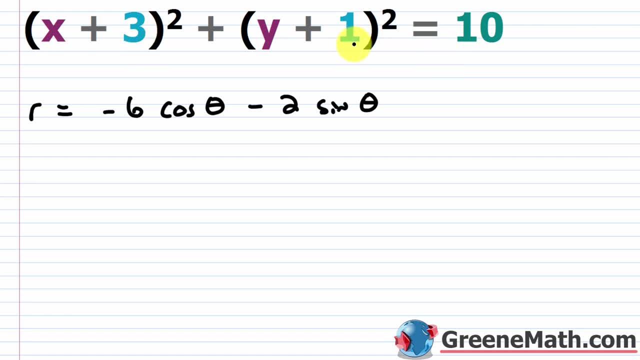 center, which would be at negative three comma, negative one. Then you would move up by square root of 10 units. You would move to the right by square root of 10 units, You'd move to the left by square root of 10 units and you move down by the square root of 10. 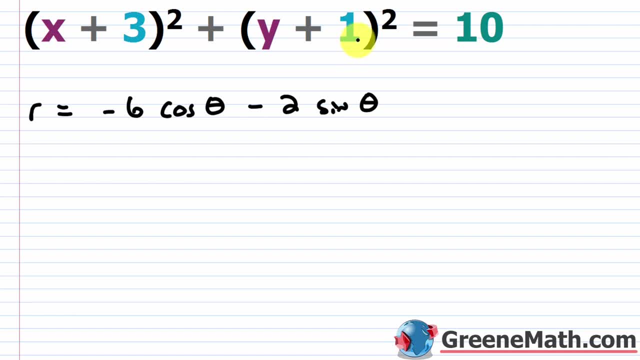 units. That would give you your four points on the circle and then you could sketch your circle. But here, because 10 is not a perfect square, we're gonna have to do a lot of estimation. Let me go ahead and put my r and my theta, and I'm going to first start with 180 degrees and the reason for. 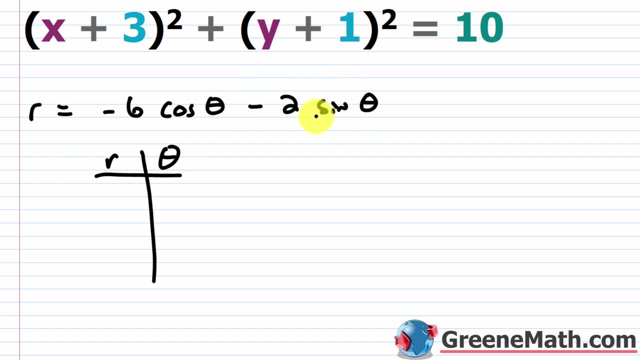 that is, I want something that's going to cancel this out completely, and I want something that's going to cancel this out completely, and I want something that's going to cancel this out completely is going to be one, So the cosine of zero degrees. is going to be one, So the cosine of 180 degrees. 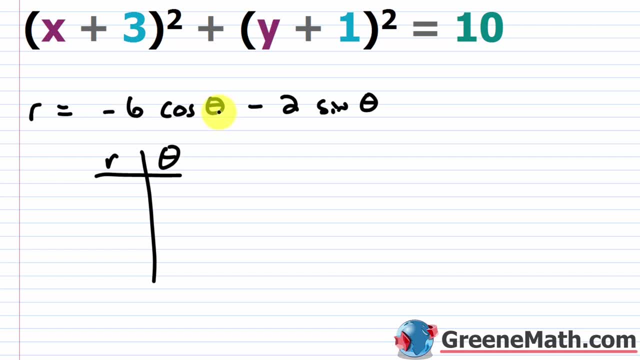 because we're flipped over. now we're going to be at negative one. Okay, so if I plugged in 180 degrees there for theta, this is gone, that's zero, right. and then this right here would be negative six times negative one, which is six. So that's one whole number value that we can get. So let me put six. 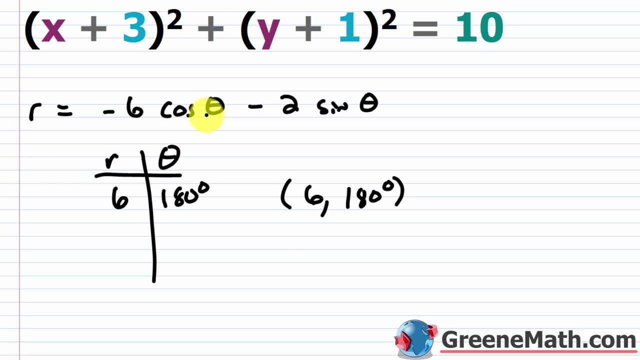 comma, 180 degrees, And then another one that we can get. If we do 270 degrees, the cosine of 270 degrees will be negative one. So that's one whole number value that we can get. So then one and then positive one degrees. that's going to be zero. so this will be gone and the sine of 270 degrees is negative one. 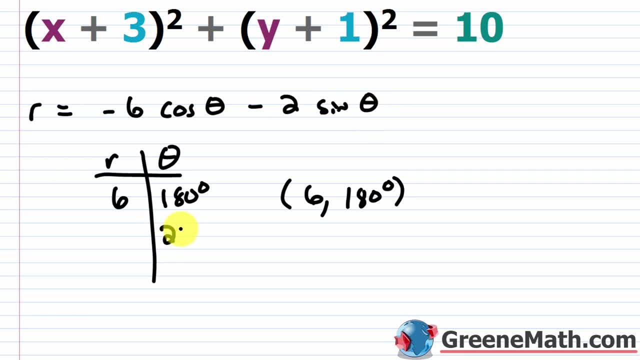 so negative two times negative. one is two. so if I do 270 degrees then basically I would have two. now for the other points. let me go ahead and put this down here as two comma, 270 degrees. I'm going to go ahead and approximate some stuff. so again, you just got to pull your calculator out. I'm going 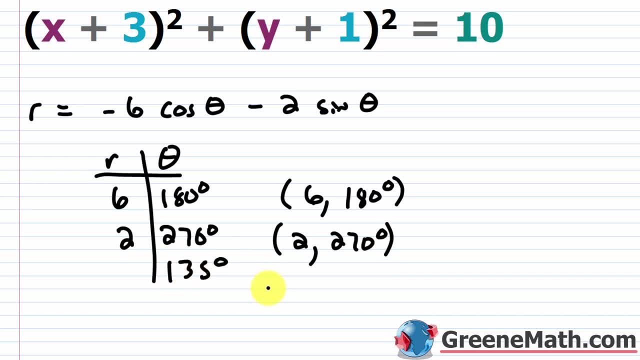 to go with 135 degrees. I think this one's going to be a little bit easy for us to work with. so if you plug this in here and here and you punch that into your calculator, you're going to get two times square root of two. so two times square root of two, okay. so two times square root of two, this is 135. 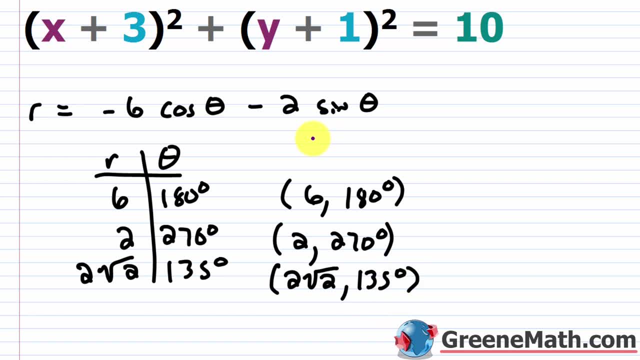 degrees. if you want an approximation for that, you could say: two times square root of two is approximately two point. let's just go ahead and say eight, three. okay, so that's close enough for me. maybe you want to get something that's a little bit closer, so you can just include more decimal. 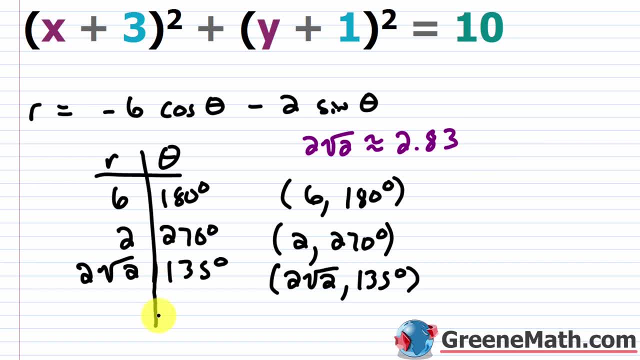 places. now let me get one more guy going here again. you take as many as you need. I'm going to go ahead and go 210 degrees here. that works out kind of nicely, so if I punch this into my calculator, I'm going to end up with three. 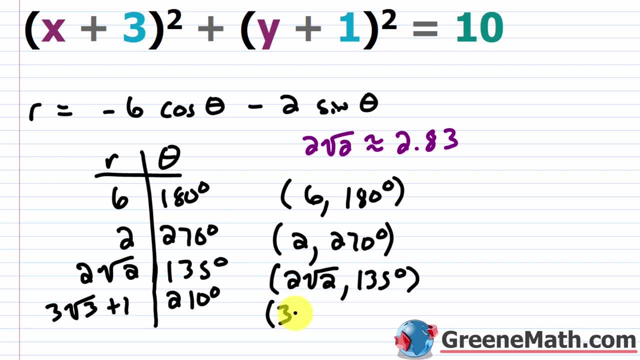 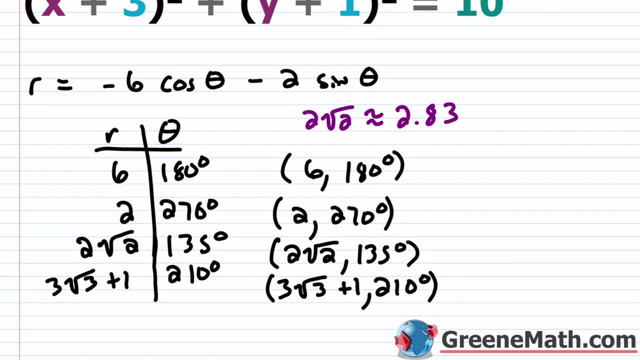 times square root of three, then plus one. okay, so three times square root of three plus one, and then 210 degrees. okay, so this one. let me go ahead and write this over here- I think I'm going to run out of rum, but I'll just put it right here. so three times square root of three plus one is: 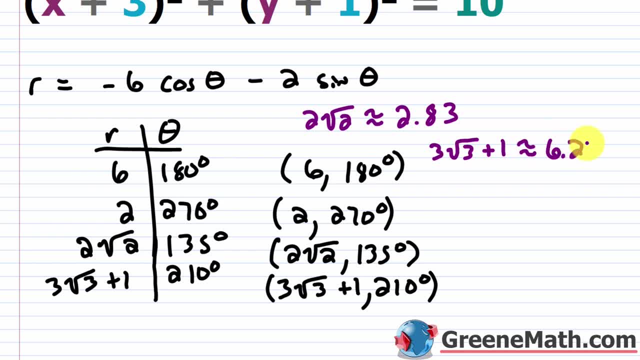 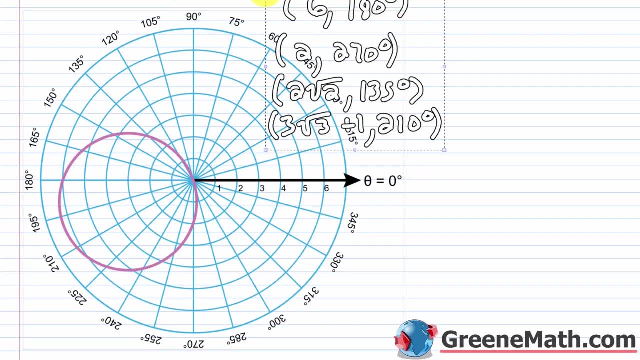 approximately. let's go ahead and say six point two. okay, so I'll say six point two. so let me grab these guys real quick. I'm going to copy this and let's come over here. I'll paste this in again. I've already drawn this with a computer which. 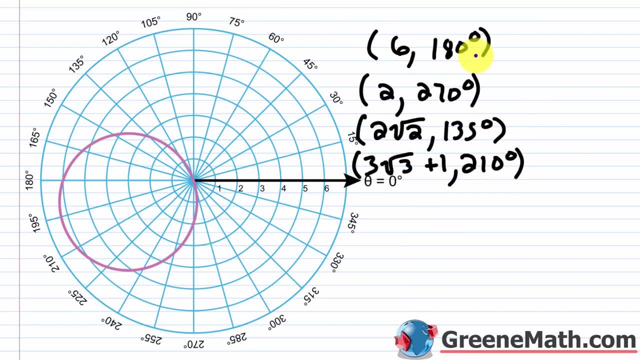 nowadays pretty much everyone does that, so I'm just going to go ahead and plot these the best that I can. so six comma 180 degrees, so I'm going to go out to a circle with a radius of six and then swing around to 180 degrees, so it's going to be right there. and then two comma 270 degrees. 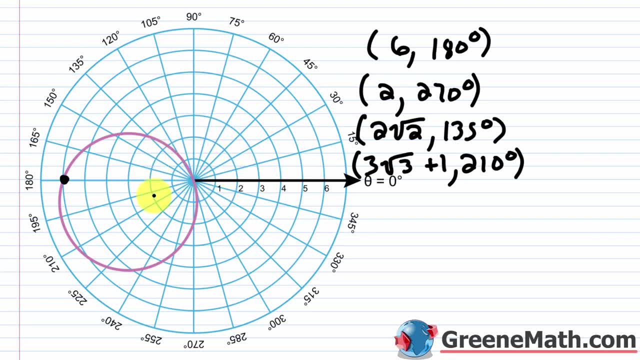 go out to a circle with a radius of two. I'm going to swing around to two hundred seventy degrees, so it's going to be right there, and then two times square root of two. we said was about two point eight three. okay, so two point eight three. so let me come out to about right. 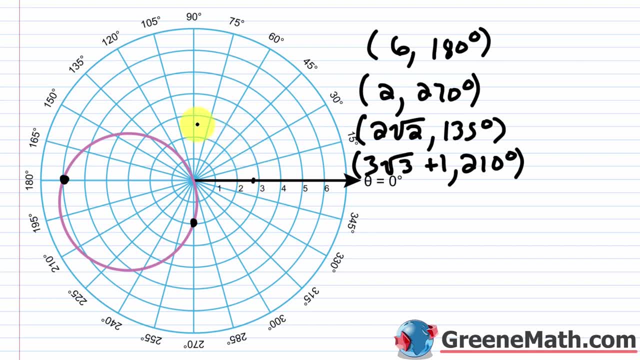 there, I'd say, and then swing around to 135 degrees. that's going to put us about. let's just say: right there again. you can't get this perfectly. we're just trying to sketch a circle. get an idea of what this looks like. if you need something perfect, you can use your ti 83 or 84, or you can use a. 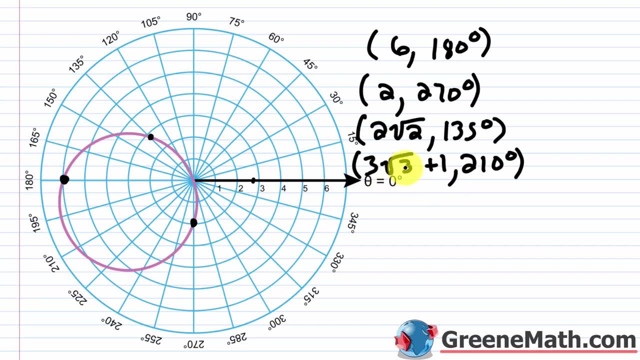 graphing calculator. so that's going to be about two times square root of two and then two times square root of three plus one. we said that was about six point two, so let's go out to this about six point two right here. and then we said that it was 210 degrees, so let me swing this around. 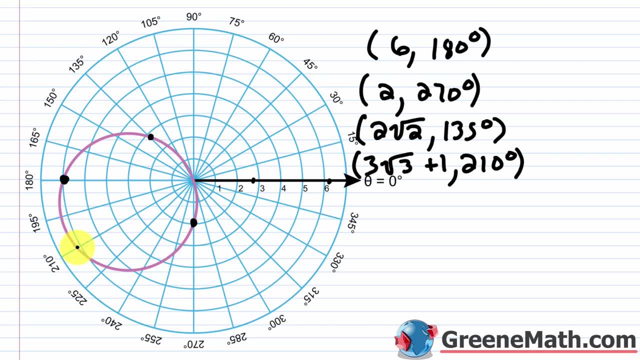 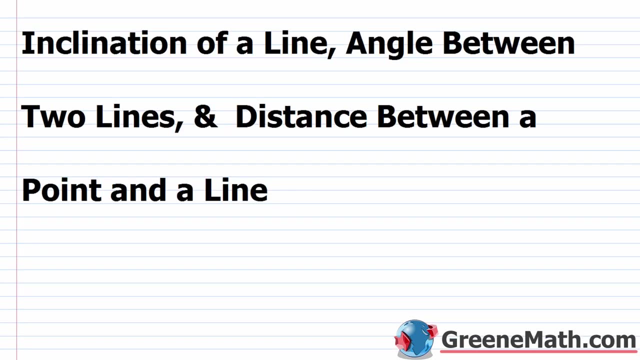 to 210 degrees. so that's going to be about right there, okay. so from those points again you could sketch your circle. it won't be perfect, but it would be close enough to get your assignment completed. in this lesson we want to talk about the inclination of a line, the angle. 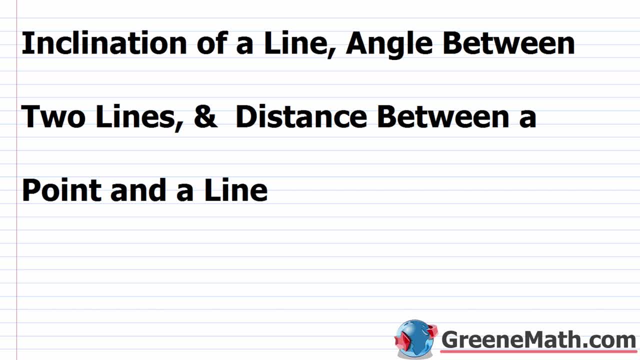 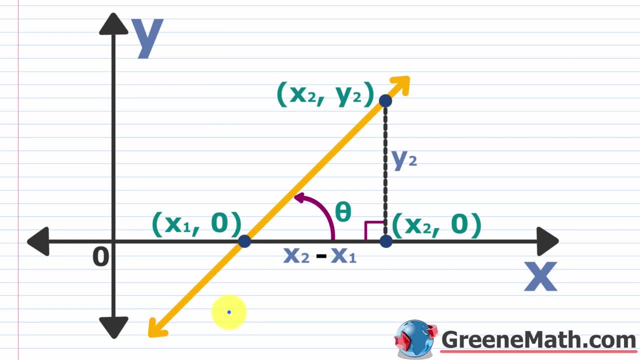 between two lines and also the distance between a point and a line. all right, so what I want to do is start out by talking about the angle of inclination. so I'm going to go through a few scenarios with you generically and then we'll look at some examples. so this is what you'll probably 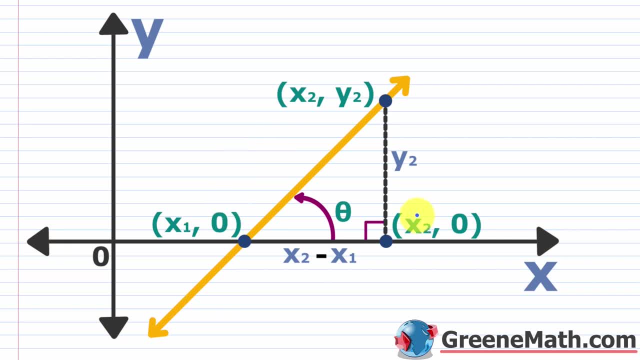 see in your textbook, and there's just a few things to go through here. essentially every non-horizontal line is going to impact the x-axis somewhere, so in this case we're looking at a positively sloped line. okay, it's going to impact the x-axis somewhere, so in this case we're looking at a. 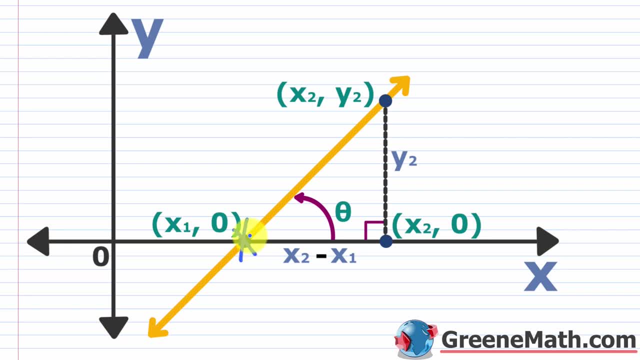 positively sloped line. okay, it's going to impact our x-axis right there, okay. so we're saying the point is x sub 1, that's your x value, and then 0 for the y value because again it's on the x-axis. you can label this as y sub 1. we're going to need that in a moment now when we talk about this angle. 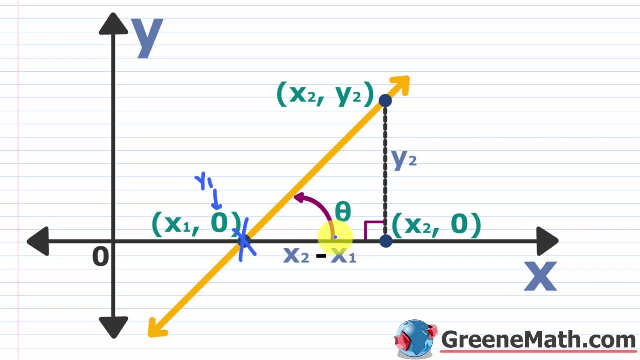 of inclination. we're considering the angle formed from the x-axis here. okay, measured counterclockwise to this line. so we're going to name this with theta. okay, so that's going to be our angle. so, with this guy right here, we're going to name this with theta. okay, so that's going to be our angle. 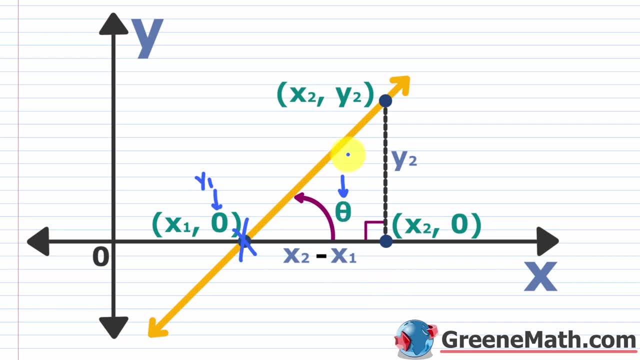 the first thing is i would consider the slope of this law. so remember, if you have two points in a line, so we have this point and then we have this point, we can use our slope form. so m, which is classically used to denote slope, is equal to remember it's rise over run. so typically we see: 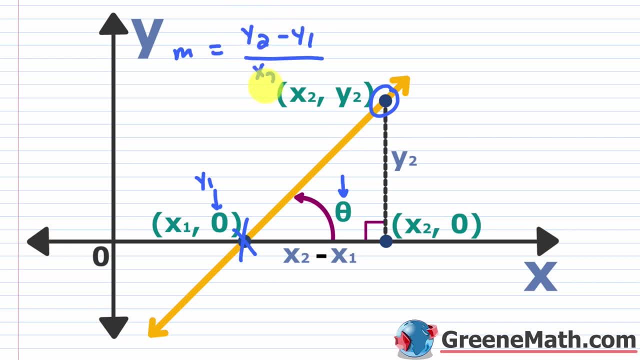 y sub 2 minus y sub 1 over your x sub 2 minus your x sub 1. okay, now, in this case, we know that y sub 1 has a value of 0, so you can just plug that in, okay, and then essentially you can simplify this. 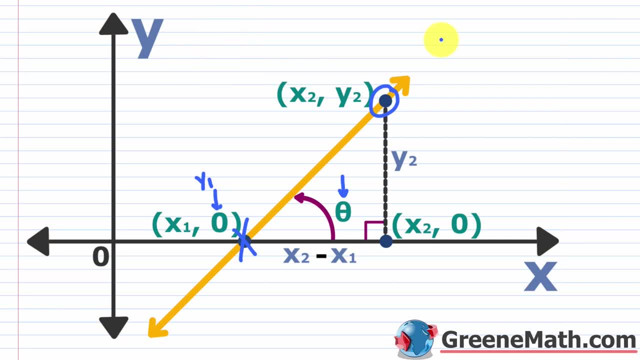 in this particular case, and then you can plug that in, okay, and then essentially, you can simplify this. let me make this a little bit neater. i'm going to say that m, our slope is going to be y sub 2 over x sub 2 minus x sub 1. okay, so that's pretty easy to understand. now the other thing we can consider: 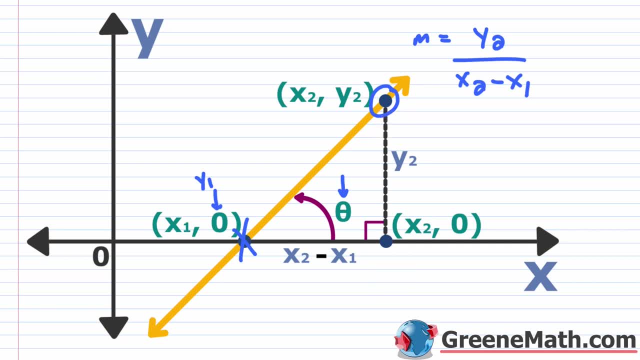 here is that we could form a right triangle. okay, so what i'm going to do is have this side right here and the length of this side, which is adjacent to our angle theta is going to be x sub 2 minus x sub 1. so this x coordinate here, whatever it is, minus this x coordinate here, whatever it is, would. 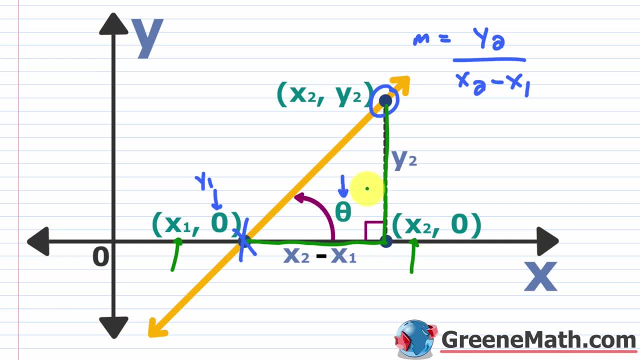 length of this side, then let's do the opposite side as well. so this is opposite of our angle, theta, and this guy has a length of y sub 2, whatever that is because you have y sub 2 minus your zero, because this point, right here again, is on the x-axis. so i want you to notice that the tangent 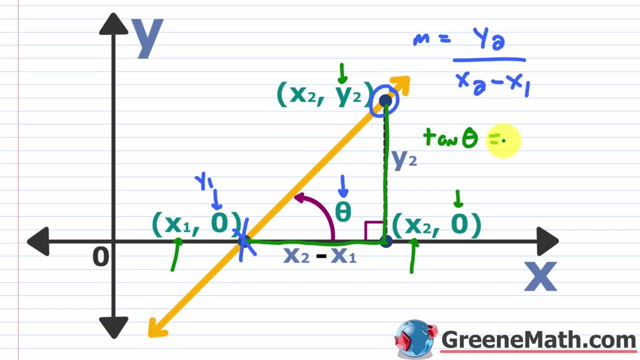 of theta. the tangent of theta is equal to what well, it's opposite over adjacent. so this is y sub 2 over x sub 2 minus x sub 1. okay, so do you see the relationship between the slope of the line and the tangent of theta? well, they're going to be equal. right m, the slope is equal to the tangent. 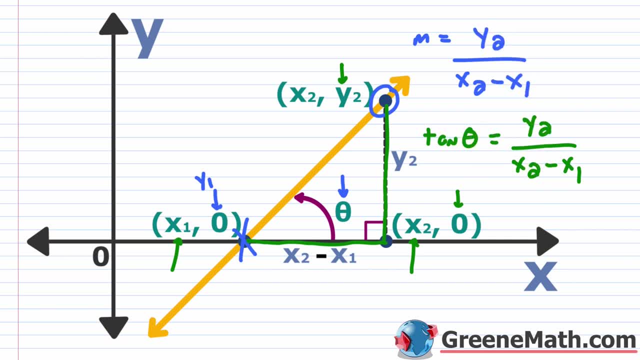 of theta, because they're both have the same definition here. so i can say that m, our slope, is equal to the tangent of theta. okay, but like all things in trigonometry, it's not always so straightforward to get your answer. all right, let's start out with the easiest scenario. this is where 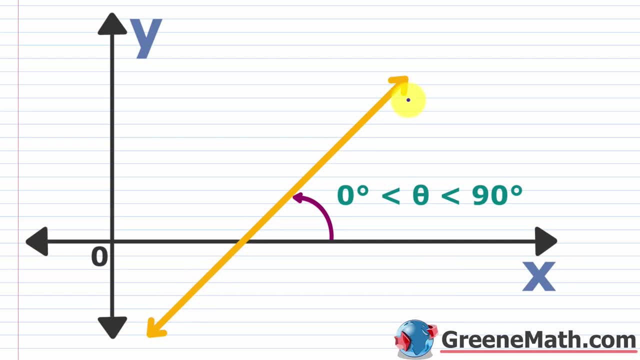 you have a positively sloped line, like we just looked at here, you're going to have an acute angle for theta, okay, so your angle of inclination will be greater than the slope of the line and the angle of inclination will be greater than zero degrees and less than 90 degrees. so in this case, 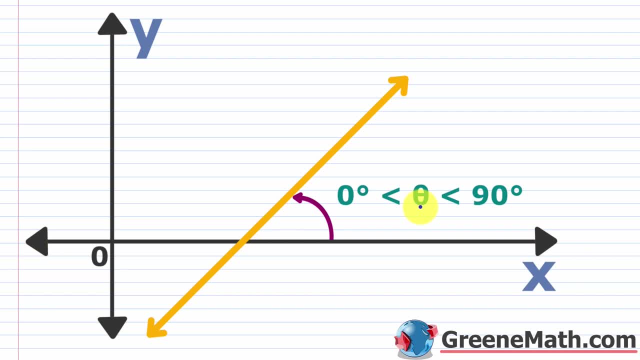 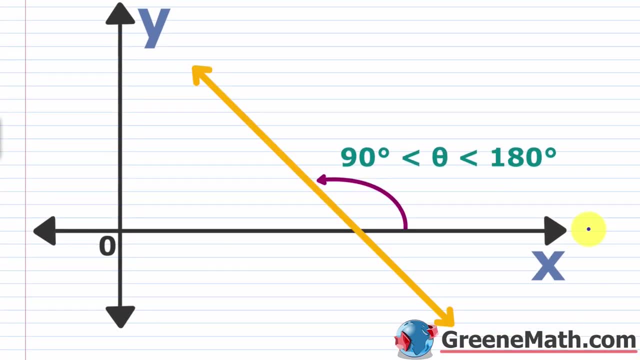 you can just plug straight in to your inverse tangent function. okay, so if you have a positively sloped line, that's all you need to do. you'll have the correct answer. okay, now the harder scenario occurs when, basically, you have a negatively sloped line, like we see here. so now you're going to have 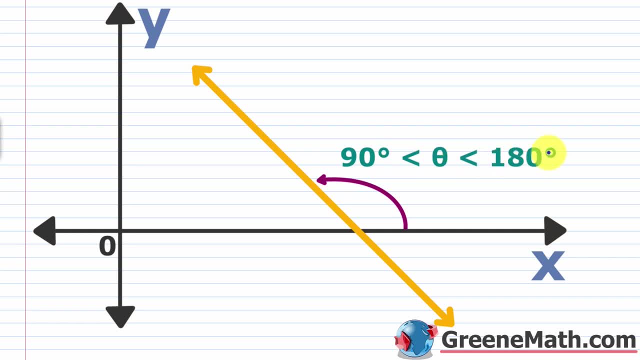 an obtuse angle. so theta is going to be greater than 90 degrees and less than 180 degrees. and for this guy you have to do more work because when you use your inverse tangent function, basically you're going to have a negative slope line and you're going to have a negative slope line, and 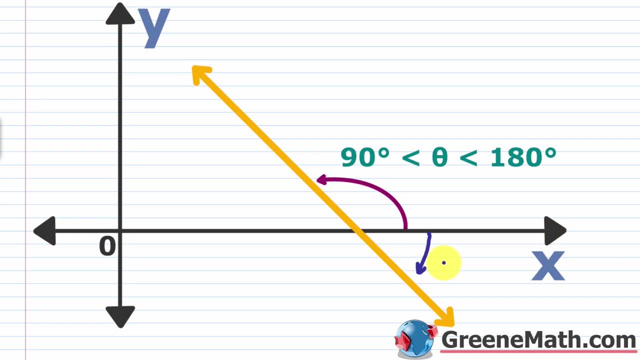 you're going to get something in quadrant four. it's going to rotate clockwise like this, and you're going to get this angle measured clockwise, okay. so what you're going to have to do is you're going to have to take that angle you get and add it to 180 degrees so that you can get this obtuse angle here. 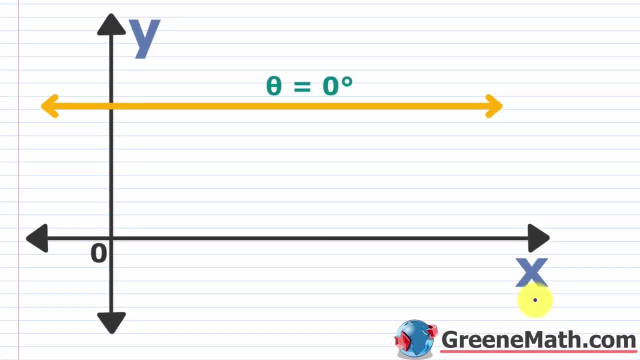 that's going to be in quadrant two, some other special case scenarios. obviously you'll have a horizontal line and a vertical line. you should know that. basically, if you have a slope of zero, right, something like y is equal to k, that's a horizontal line. the slope is zero. so theta there. 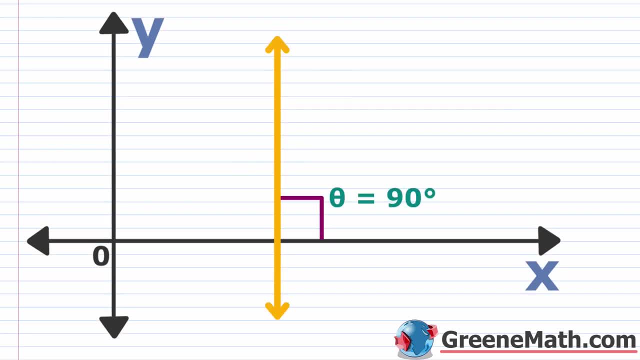 is going to be 90 degrees now. lastly, you can also get a vertical line. we know theta. here you're basically going to have a right angle. so theta, there is going to be 90 degrees and we know the tangent of 90 degrees is not defined right. we know that with a vertical line, something like x is. 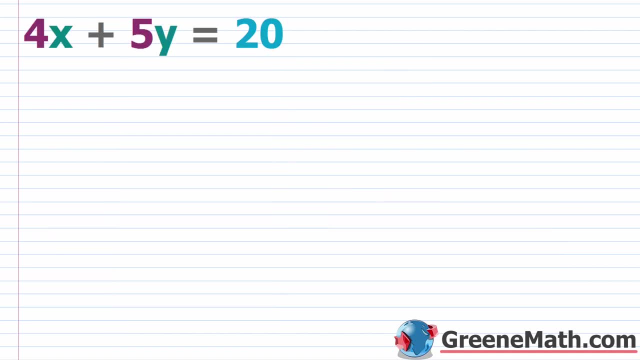 equal to k, you have an undefined slope. with all of that being said, let's go ahead and look at an example. so what i'm going to do is take this: 4x plus 5y equals 20 and put it in the slope intercept form. so y equals m, the slope times x plus b, the y. and then i'm going to take this: 4x plus 5y equals. 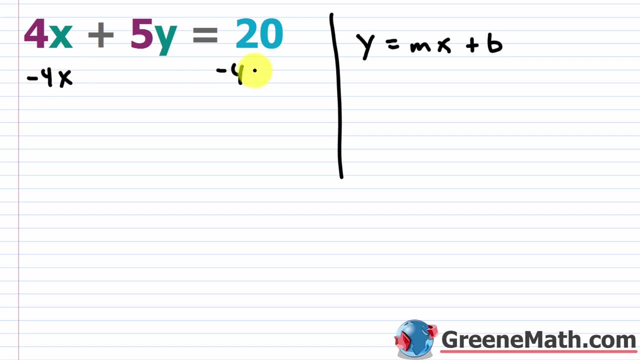 y intercept, and so i'm going to subtract 4x away from each side of the equation. that would cancel. i'll have my 5y is equal to negative 4x plus 20. divide everything here by 5 and this is going to give me that y is equal to. we'll have negative 4 fifths. okay, that's going to be my slope times x. 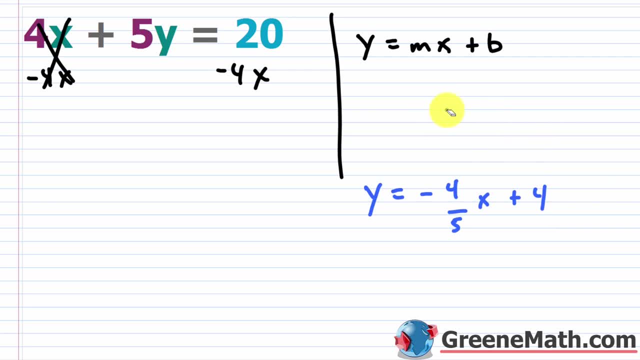 and then plus 4. okay, now, a lot of times when you first start doing these, you might want to graph it just to understand what's going on. but essentially you know that if you have a negative slope- which i have here, m is negative four-fifths, that essentially you have an obtuse angle right. so 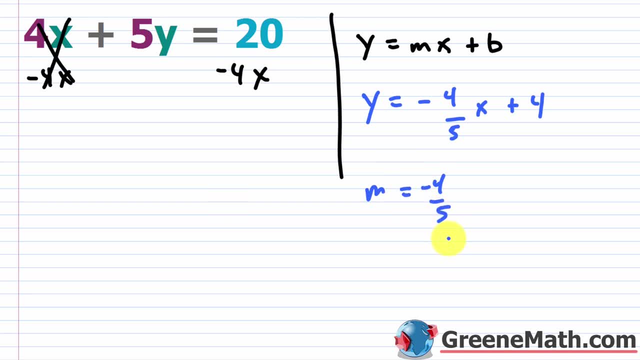 you have to do additional work with this guy and to verify that, let's just look at the graph real quick. so the slope is negative four-fifths and the y intercept is going to be at zero comma four. so let's look at the graph. so my y intercept again is at zero comma four. so that's there and my slope. 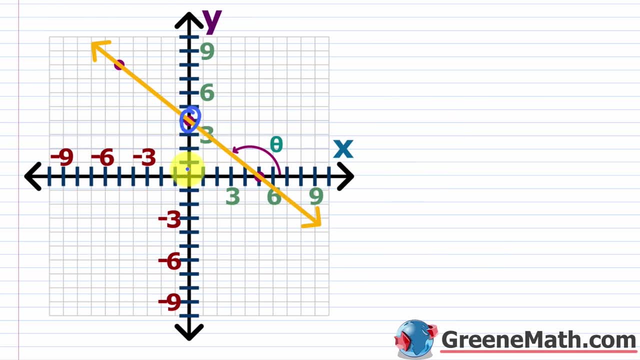 is negative four-fifths. so drop one, two, three, four to the right: one, two, three, four, five. that will give you that point right there. okay, so we're looking at this angle right here, theta. we're trying to figure out what that guy is. you can. 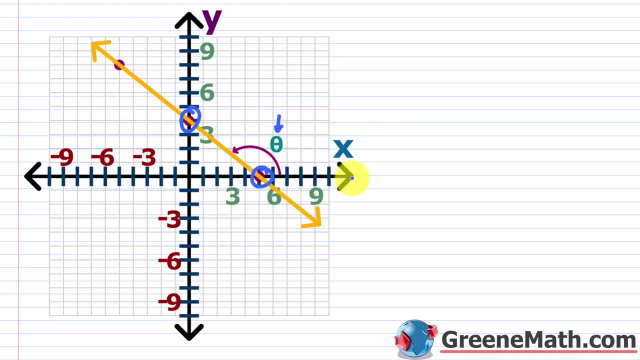 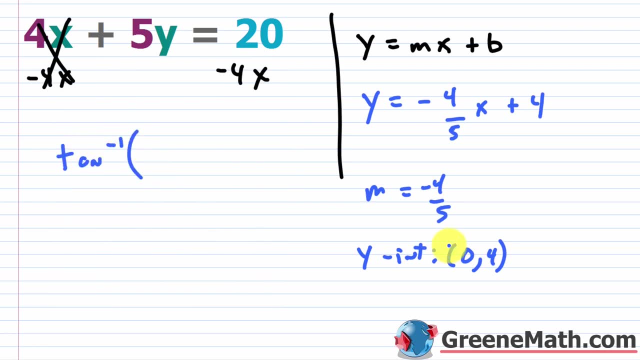 see, just by inspection, that this guy is going to be an obtuse angle. okay, so we know we're going to be in quadrant two. so again, what you want to do is you want to say the tangent inverse of this guy, so negative four-fifths. just punch that into your calculator. you're going to get approximately. 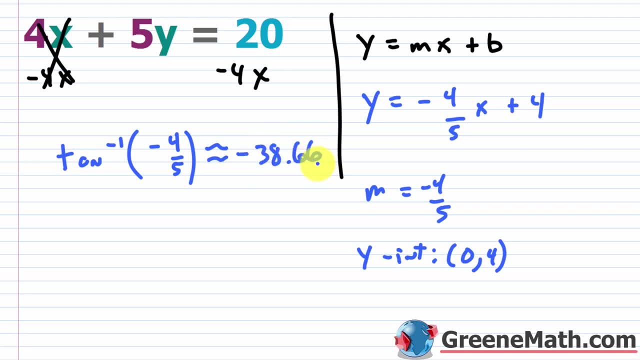 i'd say negative 38.66. okay, let me put degrees there to be specific. now, once you have this again, what you want to do is you're going to want to do. is you're going to want to do is you're going to? because you're looking for your angle in quadrant two. this is giving you something in quadrant four. 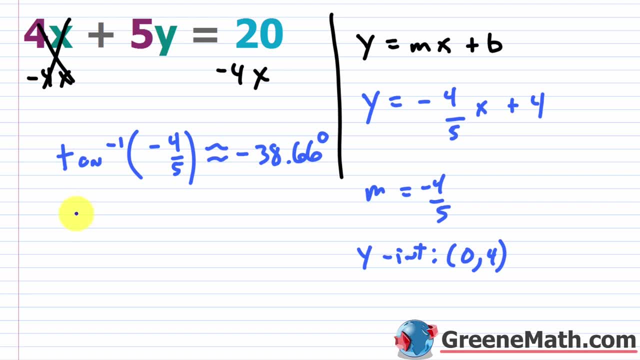 rotating clockwise, okay. so what i want to do is i want to say, okay, 180 degrees plus this negative 38.66 degrees is going to give me, i'll say, about 141.34 degrees. okay, so this would be my angle of inclination. obviously this is an approximation and i'll say theta is approximately 141.34 degrees. 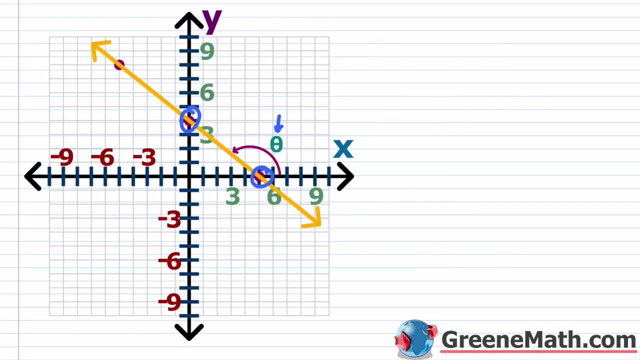 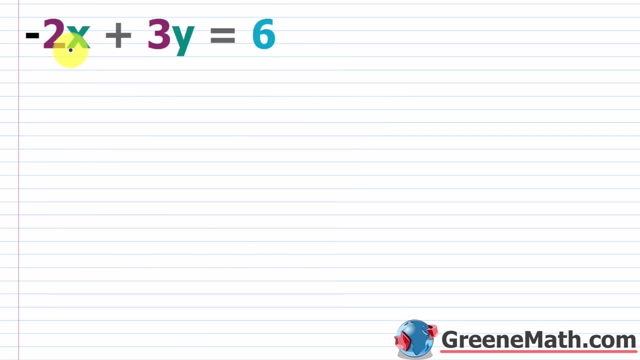 141.34 degrees. now what i would do when i first start this is go back to your picture- if you made a graph- and just say, okay, is that about 141.34 degrees? yeah, that looks about right. so i'm going to put approximately 141.34 degrees. all right, let's try another. so we have negative 2x plus. 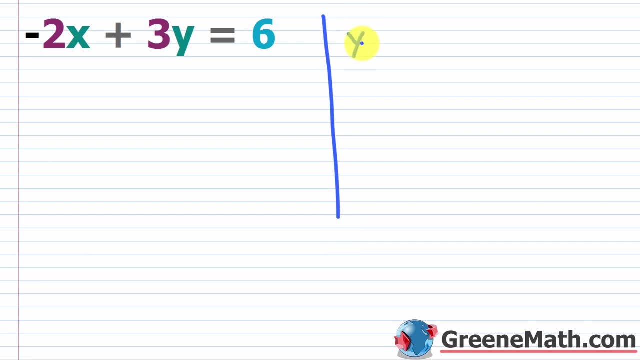 3y equals 6. again i'm going to put this in slope intercept form. so y equals mx plus b. so basically i would have if i add 2x to both sides, then what i would have is a negative 2x plus 3y equals 6. 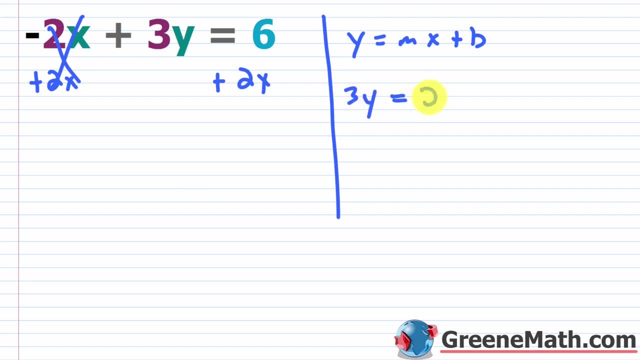 this canceling over here. i'll have 3y is equal to 2x plus 6, and then i'm going to divide both sides by 3, okay, and i'll have y is equal to two-thirds. okay, that's going to be my slope times: x plus 6. 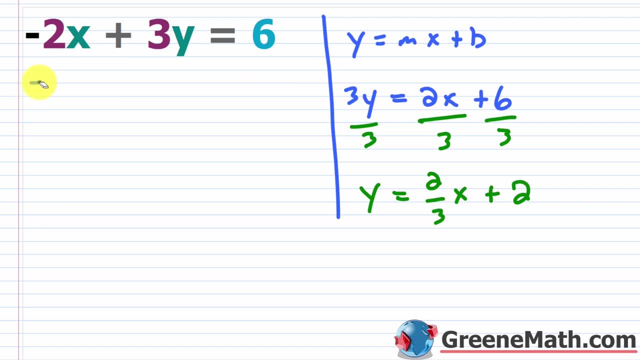 divided by 3 is 2. okay, so your slope- let me get rid of this- your slope m is going to be two-thirds and your y intercept, your y intercept, is going to occur at 0 comma 2. okay, so if we look at the graph of this guy, 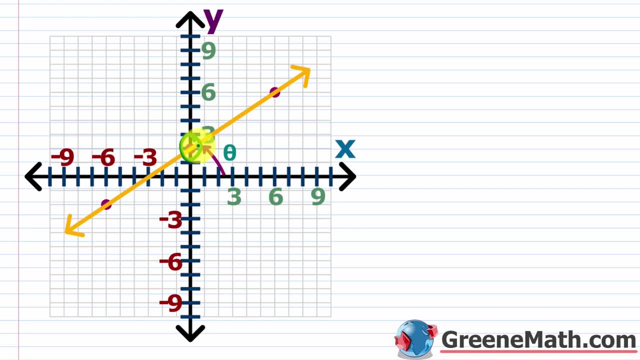 you would say: okay. well, your y intercept is at 0 comma 2, your slope is two-thirds. so up 1, 2 to the right, 1, 2, 3. okay. so right there. up 1, 2 to the right, 1, 2, 3. so right there. okay, so you have. 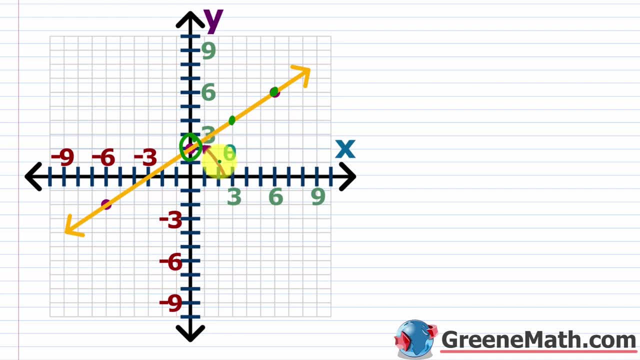 some points you can draw that line again. we're looking for this angle, theta. you can see this is an acute angle, right? so basically, i would want to say the tangent inverse of let's go ahead and say two-thirds. this is approximately, i'll say, 33.69 degrees. 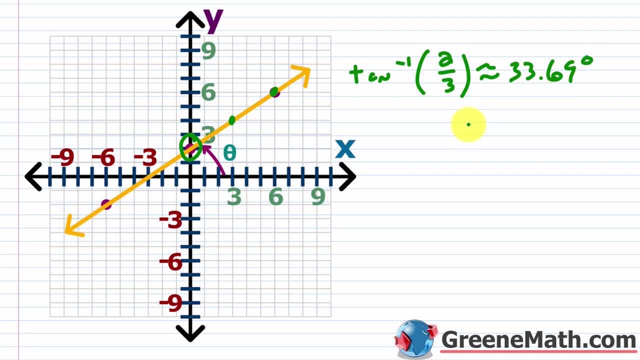 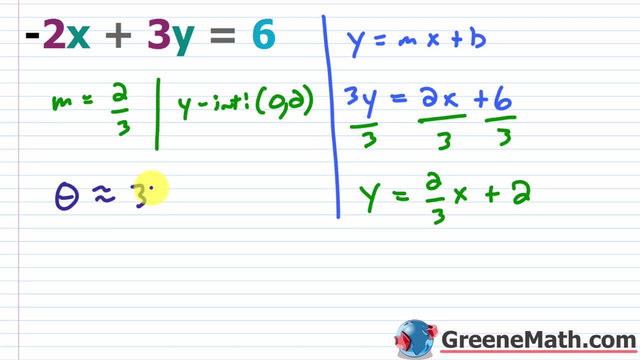 and we don't need to do anything else here because this guy is in quadrant one right. so basically i can say this is approximately 33.69 degrees. if you want to go back to where we had our problem, you could say: theta again is approximately 33.69 degrees. so when you have 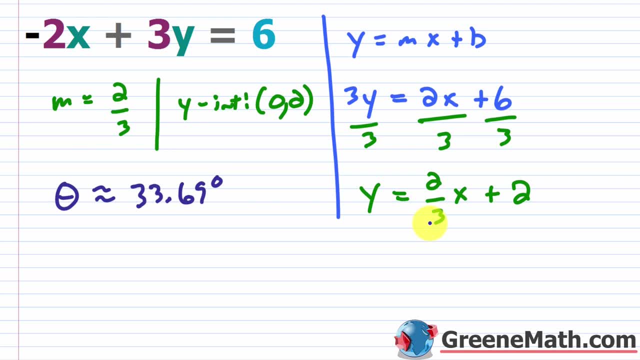 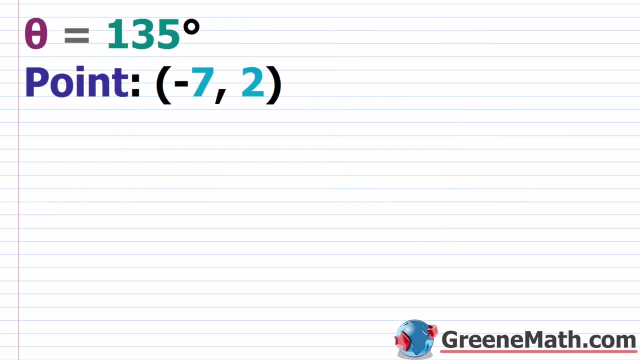 a positively sloped line like this. it's really really easy. just plug this into your inverse tangent function and you're done. you don't have to do any extra work. okay, let's look at one of our that is in reverse. so now we're given our angle of inclination, our theta is 135 degrees and we're 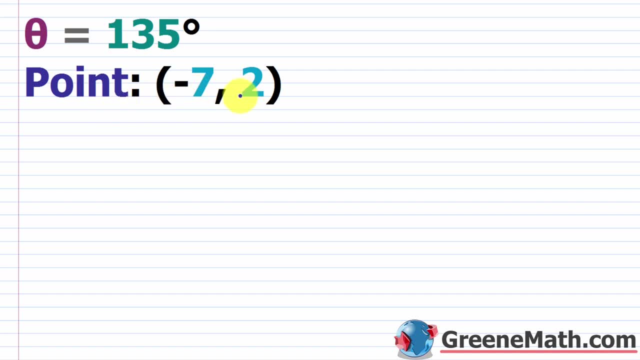 given a point on the line which is negative, 7 comma 2, and essentially we want to write the equation of the line, and so if we wanted to do this, the first thing is we need to figure out the slope right. so the slope is going to be what? remember, m is equal to the tangent of theta. well, 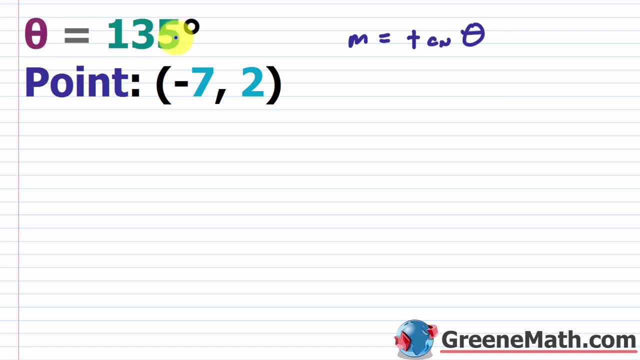 i have theta. so if i take the tangent of 135 degrees, what would that give me? so my tangent, my tangent of 135 degrees, is equal to. i'll go ahead and say m, which is equal to negative 1. okay, so i know the slope is negative 1, so let me erase this and put negative 1 here. you can get rid of this now if i. 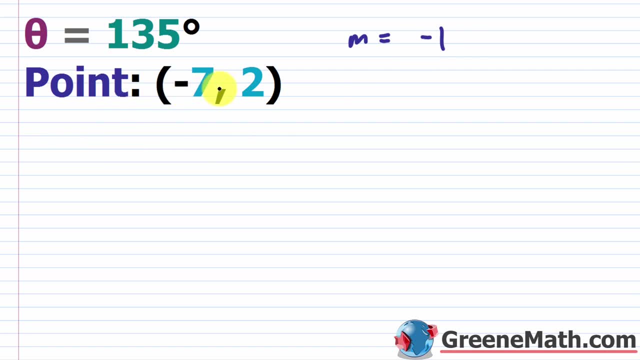 have my slope, which in this case is negative 1, and i have a point of the line. let's call this x sub 1 and then y sub 1. well, i can plug into something called point slope, right? so y minus y sub 1 is: 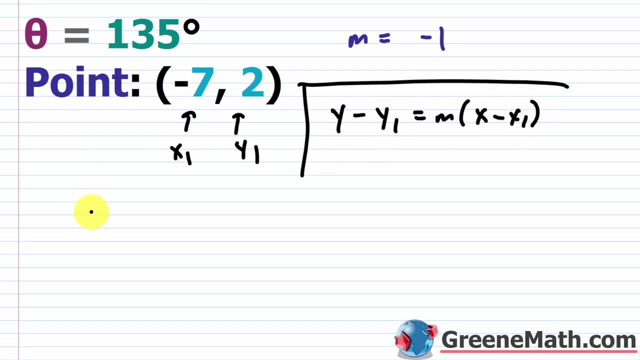 equal to m times the quantity x minus x sub 1. so here y minus my y sub 1 is 2, is equal to m, which is negative 1 times the quantity x minus x sub 1 is negative. 7 minus the negative 7 is plus 7. now you can solve this for y and put it in slope intercept form. 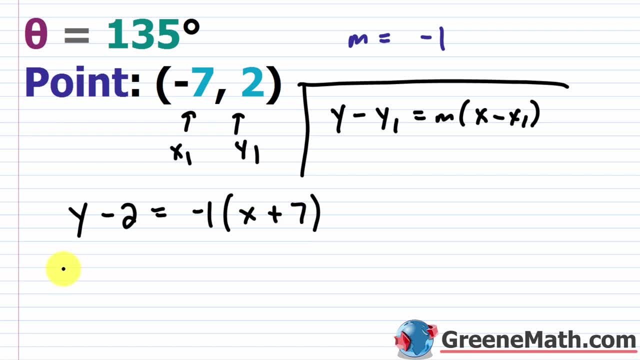 you might also be asked to put it in standard form, so just get with your instructions. so y minus 2 is equal to. this would be negative x and then minus 7. let me add 2 to both sides of the equation. let me erase this and i'll go ahead and say that our equation is: y is equal to. we'll say: 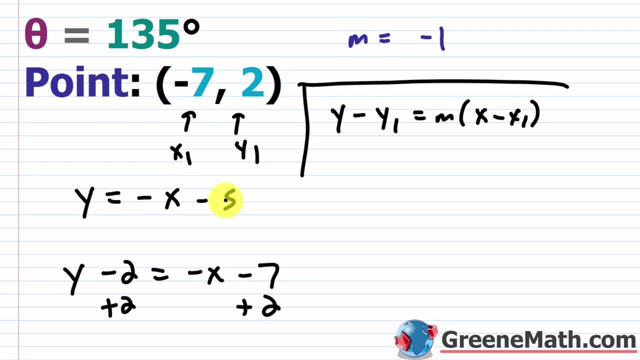 that it's negative x, and then we'll go ahead and say minus the equal to x. so y sub 1 is 2 is equal to minus 5.. Okay, so that's your slope intercept form of the line, If you want to look at this. 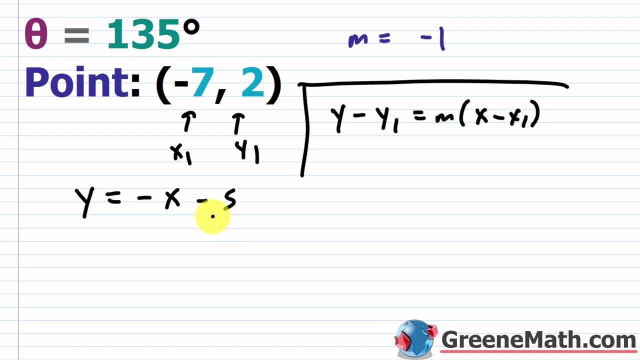 graphically, your y-intercept would occur at 0 comma negative 5, and your slope would be negative 1. So your y-intercept would be at 0 comma negative 5, so that's right there and your slope is. 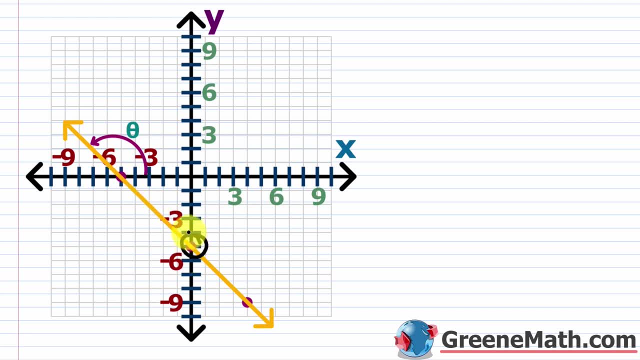 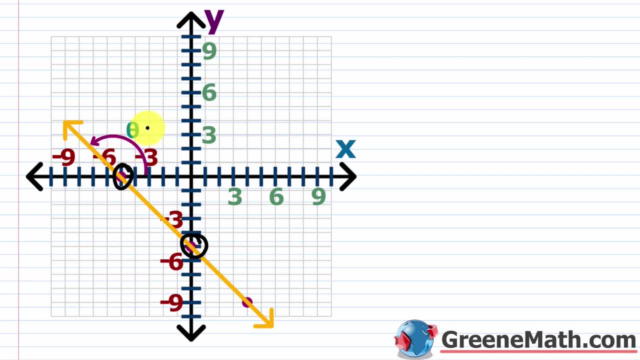 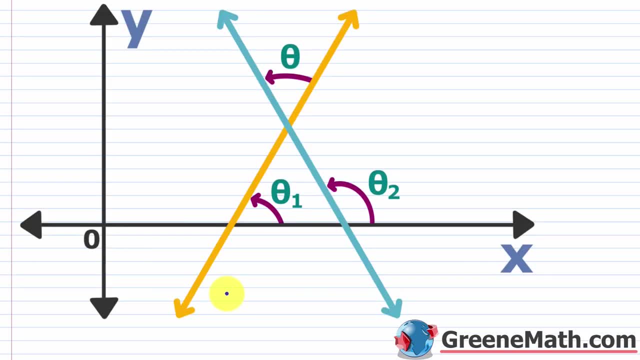 till. you get to this point here And you can see. we have this angle theta here, which is going to be equal to 135 degrees. All right, so what we want to do now is talk about the angle between two lines. So if you have two lines in a plane, they're either going to be parallel lines, 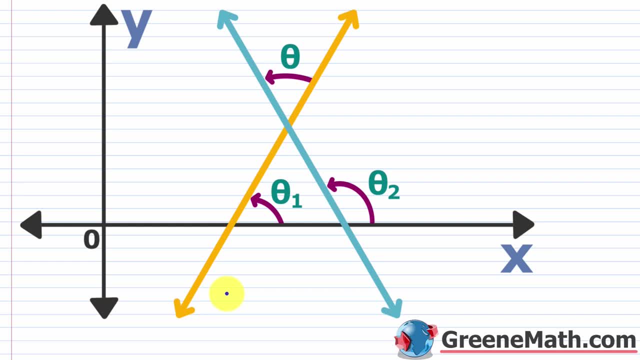 in which case they'll never intersect, or they'll be non-parallel lines, and in that case they will intersect at some point. Okay, so the case we would talk about here today will be non-parallel lines, obviously because we need some point of intersection, and also they're not. 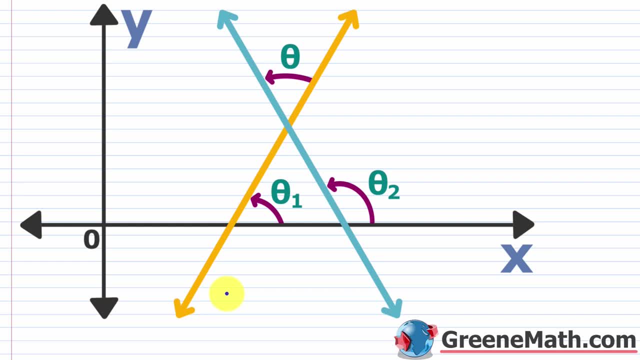 going to be perpendicular lines because we don't want them to meet at 90 degree angles. Okay, so we're talking about the other situation, So I have a little image here which I want to focus on. So you'll see that this point of intersection here 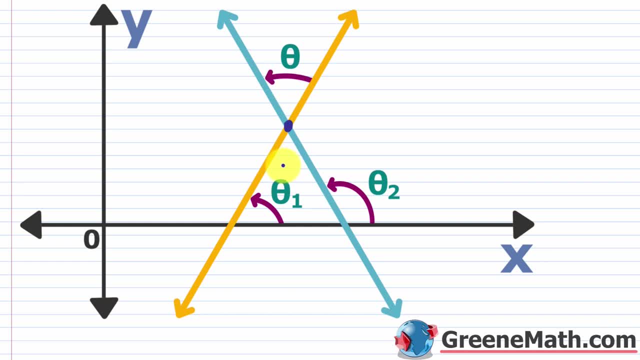 forms two pairs of opposite angles. So you have these acute angles, so you have this one and you have this one, right, So those would have the same measure. And then you have these obtuse angles, so you have this one, and then you have this one, right, So those would be of the 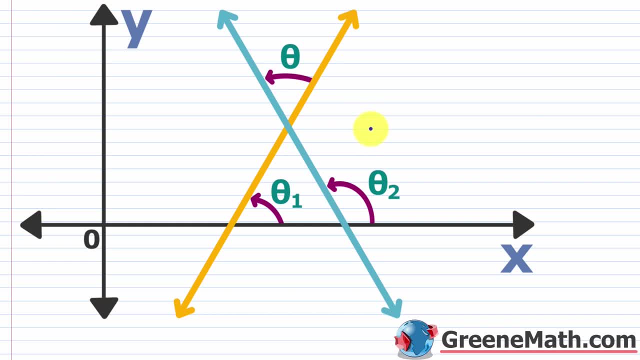 same measure as well, What we're going to focus on when we say the angle between two lines, this acute angle right here, which I'm calling theta, Okay. so we're going to be focused on how to find theta. So theta is equal to what? Well, to come up with a little formula, we're going to 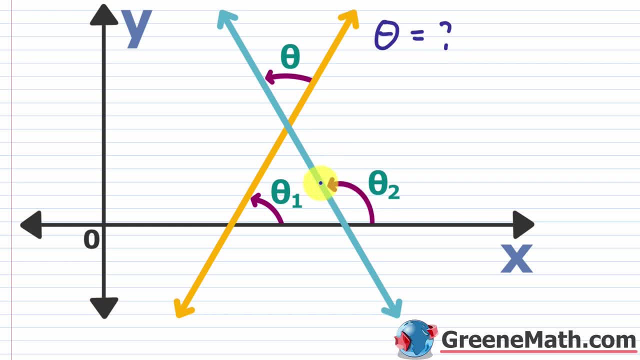 start off with this scenario, and this won't work in every scenario, so we're going to have to adjust our formula just a little bit. Okay, so we're going to say that this blue line here is a negatively sloped line, okay, And so the angle of inclination here, theta, sub 2, we know that. 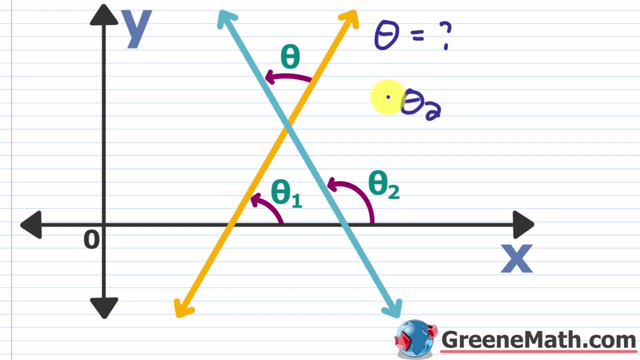 that would be an obtuse angle, right? So we can say that theta sub 2 would be an obtuse angle. is greater than 90 degrees and less than 180 degrees. So we know this. Then this orange line is positively sloped, so we know theta sub 1, the angle of inclination. there is an acute angle. So 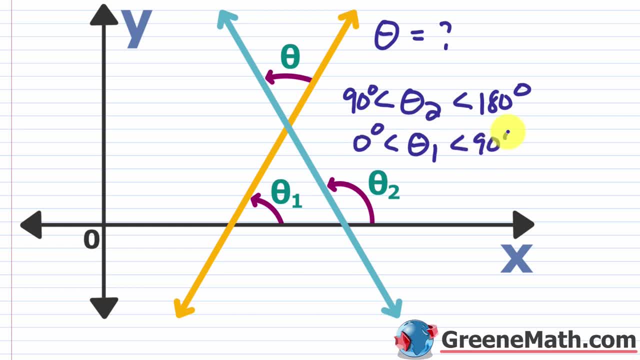 theta sub 1 is greater than 0 degrees and less than 90 degrees. So based on this, we know that theta sub 1, in this case, is going to be less than theta sub 2,. okay, So we can say: let me erase. 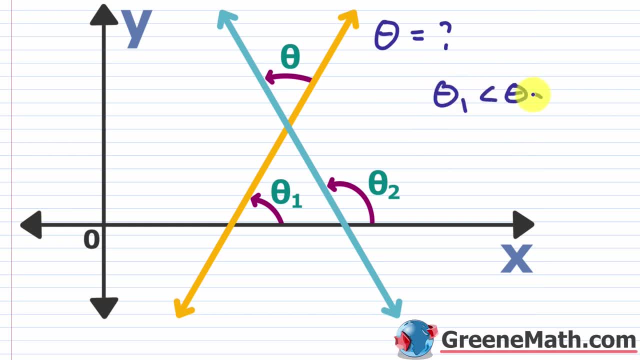 this, I'll just say that theta sub 1 is less than theta sub 2,. okay, So that's for this case. Now, because these lines are not going to be perpendicular, I can say that theta sub 2,, which is the bigger angle here, minus theta sub 1,, which is the smaller angle, is going to be. 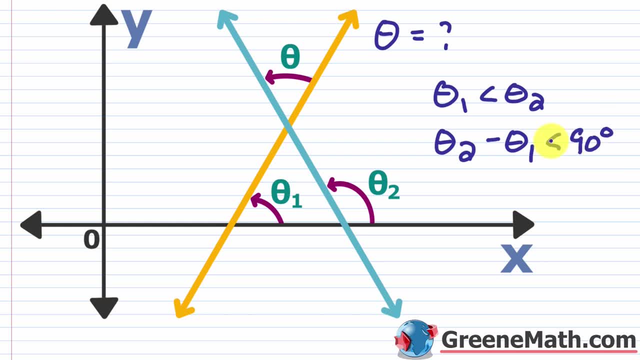 strictly less than 90 degrees, Because if this was equal to 90 degrees, these guys would be perpendicular. okay, So we're talking about these two assumptions to make what I'm about to say work. If these two assumptions don't hold, we're just going to change our formula up just a little bit. 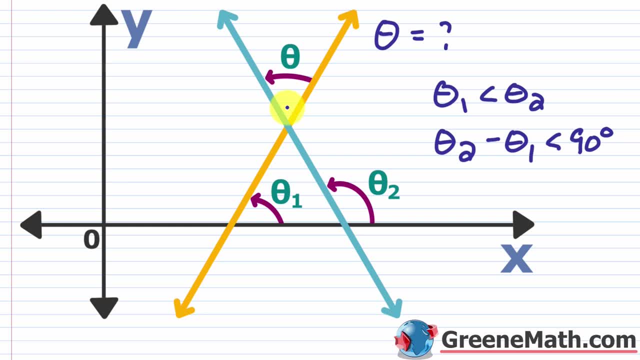 We're going to do this with using the absolute value operation, but we'll get to that later on, okay? So what I'm going to say is that theta sub 1 is less than theta sub 2, and theta sub 2 is less than. 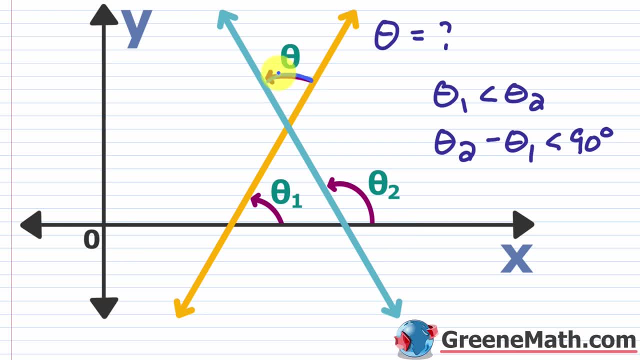 theta sub 1.. So what I'm going to say here is that if I want this angle here, okay, I can find it by first getting this larger angle- okay, Think about that- And then just subtracting away the smaller angle. So, in other words, I'm just finding this piece right here, So it's going to be the 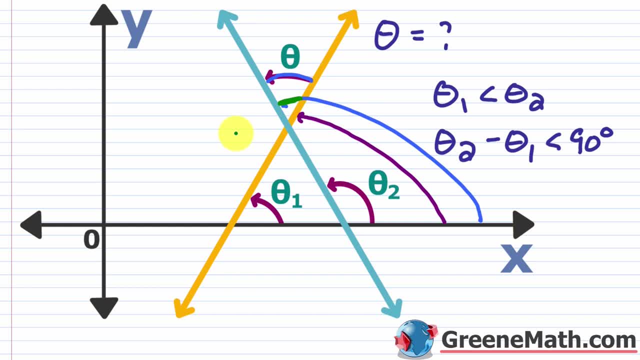 theta sub 2, okay, minus the theta sub 1.. So this is equal to, we'll say, theta sub 2 minus theta sub 1, okay, So that's for this case. right here, We're going to use this to derive a little simple. 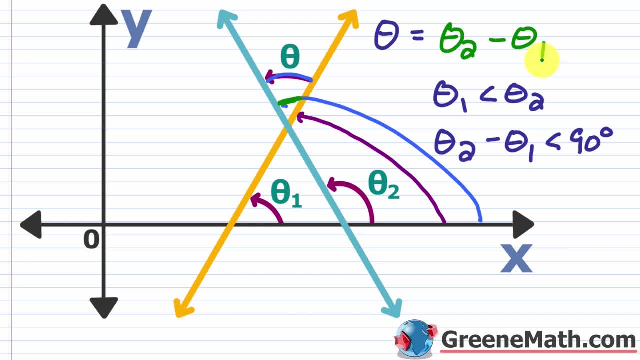 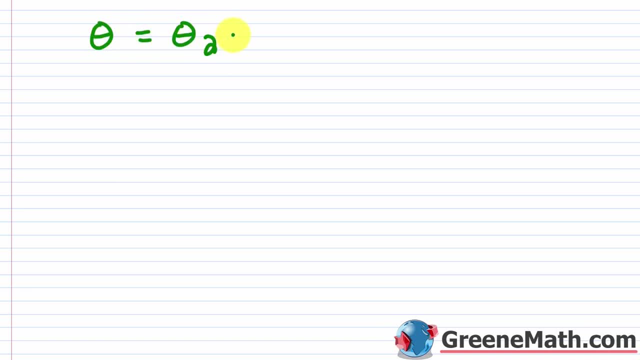 formula and then I'll show you how to correct it from here. So let's go ahead and do that For other scenarios. okay, So let's go down and say that we have theta is equal to theta sub 2, remember, this was our bigger angle minus our theta sub 1, which was the smaller angle. okay, 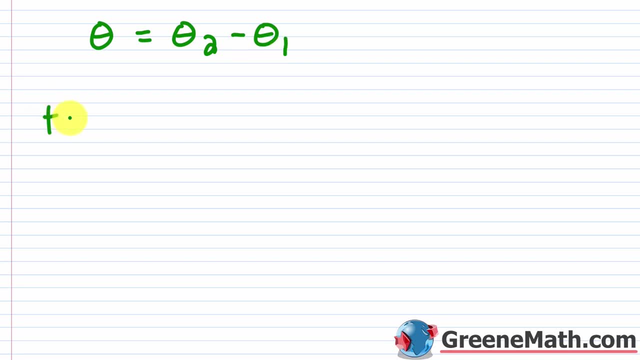 So what we're going to do here is we're going to take the tangent of each side. So I'm going to say the tangent of theta is equal to. we're going to say the tangent of this theta sub 2 minus this theta sub 1.. Remember, you cannot distribute this in. you have to use an identity. So if we go back, 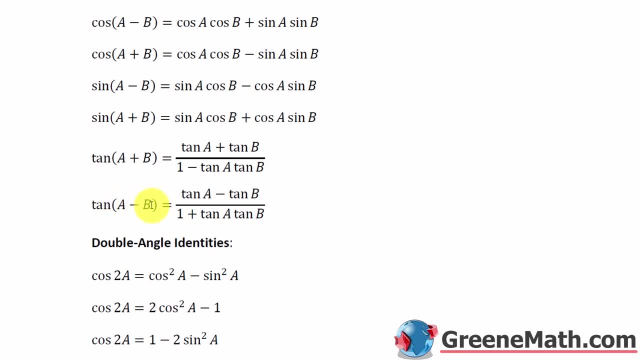 to our sum and difference identities, we see the tangent of theta sub 2 minus theta sub 1.. So what we're going to do here is we're going to take the tangent of a minus b- is the tangent of a minus the tangent of b over 1, plus the tangent of a times the tangent of b. okay, So we're just 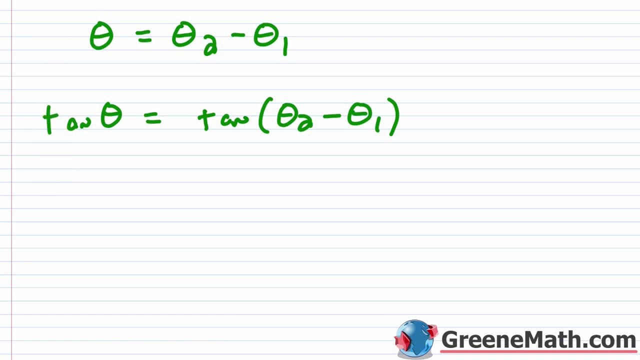 going to follow that And we're going to say that this is basically equal to: we'll do the tangent of this first guy, theta sub 2, minus the tangent of this second guy, theta sub 1.. This is over. we're going to do 1 plus we're going to multiply the two together. Now your book is going to. 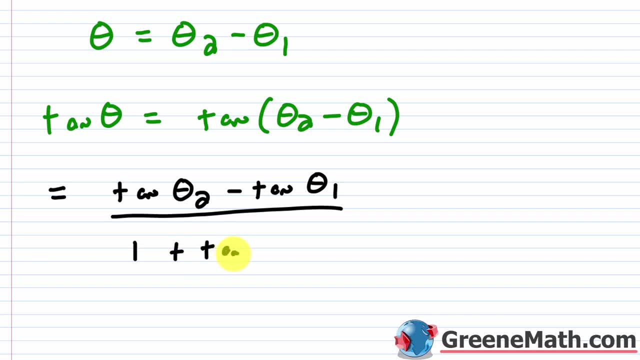 change the order of this. This is up to you. So I'm going to go: tangent of theta sub 1, times the tangent of theta sub 2,. okay, With your identity handout, it's tangent of theta sub 2 times tangent of theta sub 1, but you can multiply in any order, you'll get the same. 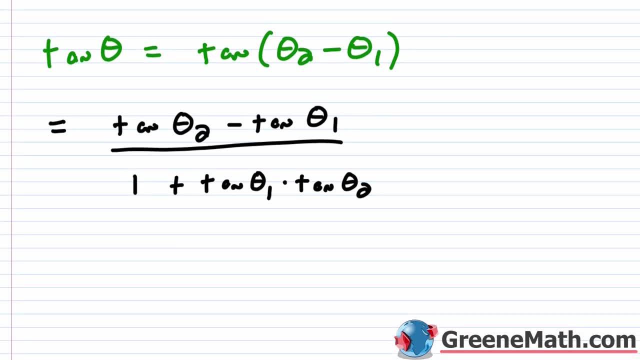 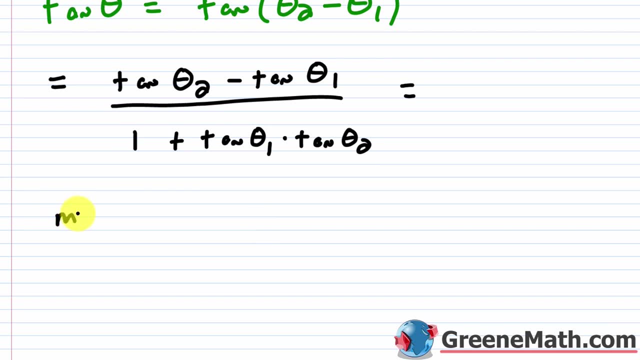 answer, so it doesn't matter, okay. So let's go down a little bit. We're going to keep this going From here. I'm going to make some other substitutions. I want you to recall that we say that our slope of a line m is equal to the tangent of our angle of inclination, which we 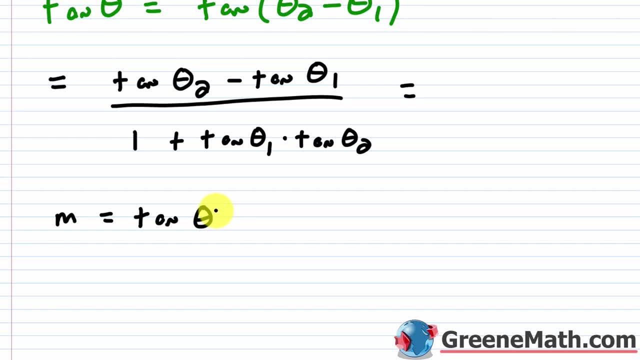 call theta. okay. So now let's say I have two different lines, So I have theta, theta, theta. two different slopes and two different angles of inclination. okay, So I'm going to say that this is m sub 1, and this is going to be theta sub 1, and this is m sub 2, and this is going to. 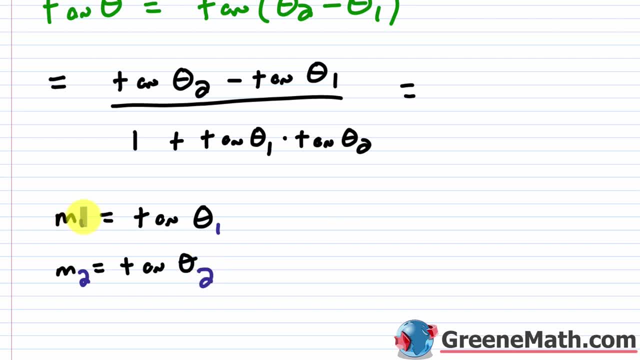 be theta sub 2.. So what I'm going to do now is just plug some things in. Since m sub 1 is equal to tangent of theta sub 1, well, where I see a tangent of theta sub 1, I can just plug in an m. 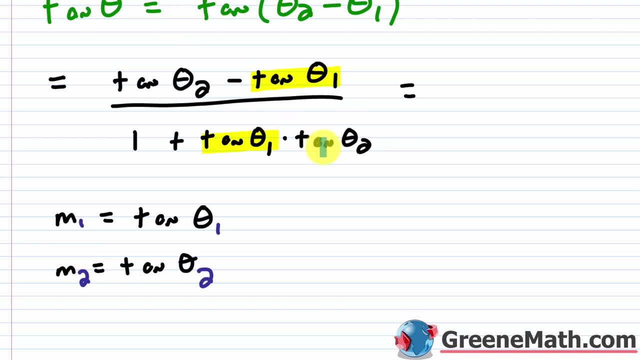 sub 1.. And then similarly wherever I see a tangent of theta, sub 2,. so here and here I can just plug this over a little bit so I can fit everything on the screen. I'm going to say that this is my m. 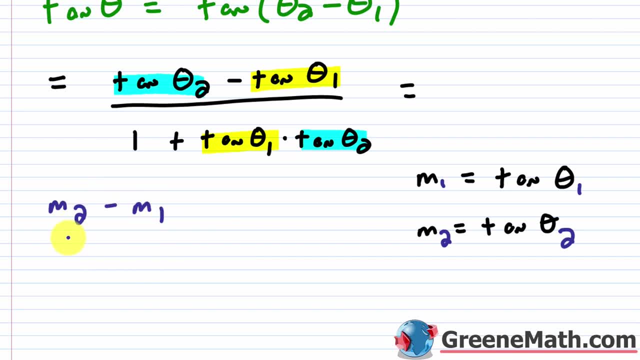 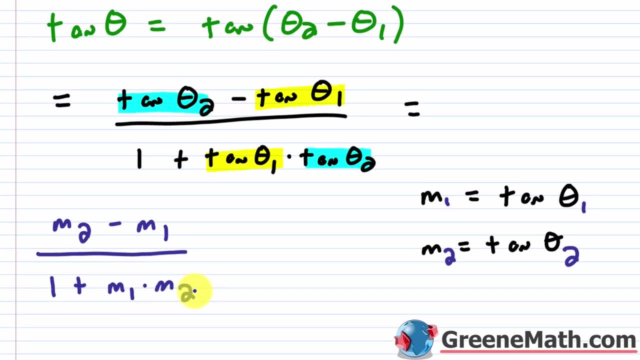 sub 2, and then minus my m sub 1, okay, And then over 1 plus, I'm going to multiply them together, so m sub 1 times m sub 2, okay. So let's talk about correcting this, Essentially because I 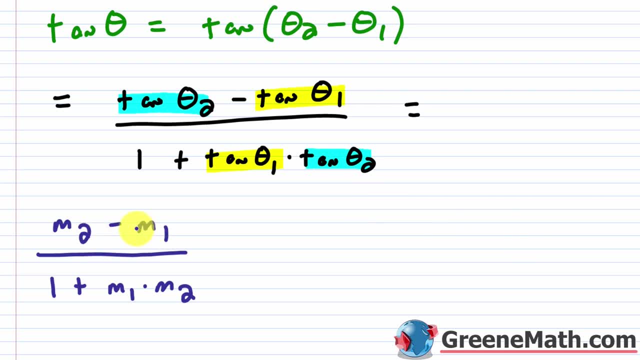 want to end up with an acute angle, okay, And I don't want to have to worry about which slope is going to get put as m sub 1, or which slope is going to get put as m sub 2,. I can just use absolute value bars here, okay. The reason this works is that, basically, if you 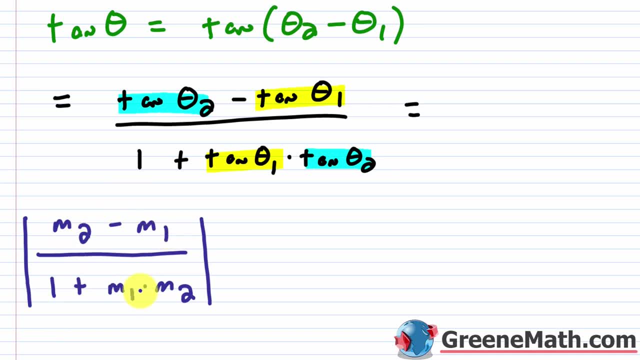 do this in the wrong order, you're going to end up with a negative inside of here, okay, And so you don't want that right. Remember: if you do the inverse tangent with a negative, you're going to get something in quadrant 4, okay. If you add 180 degrees to that, you're going to get the obtuse. 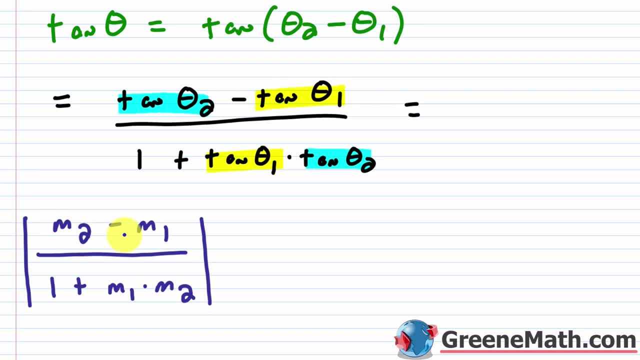 angle that's between these guys and you want the acute one, okay. So you just want to make sure you use the absolute value bars so that whatever answer you get, just make it positive, okay. And when you make it positive, when you do your inverse tangent function. 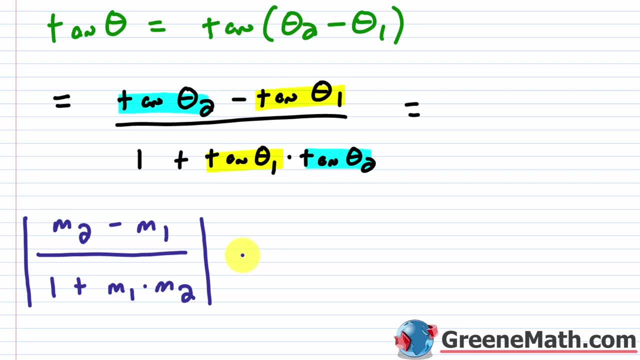 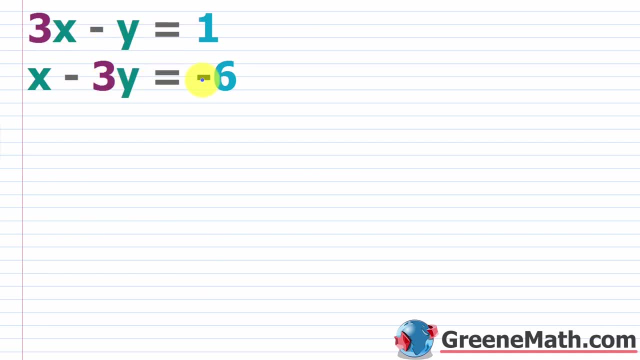 you're going to end up with the answer in quadrant 1, which is your acute angle between the lines. All right, so we have 3x minus y equals 1, and x minus 3y equals negative 6.. So I like to put these in slope intercept form. I also like to graph them. So let's go ahead and. 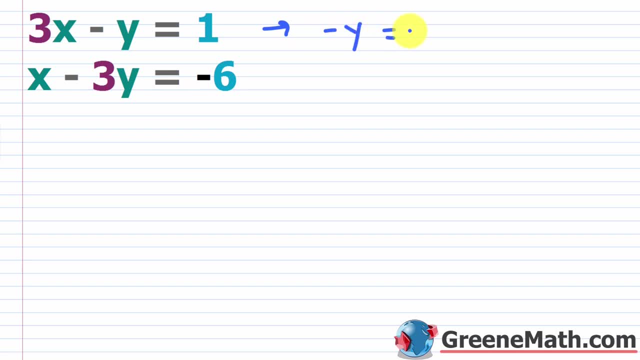 say: this is going to be what, This is negative y, and then I'll say: equals negative 3x plus 1.. I just subtracted 3x away from both sides and then basically I could multiply everything by negative 1, so that would change this sign, this sign and this sign. okay, So in slope. 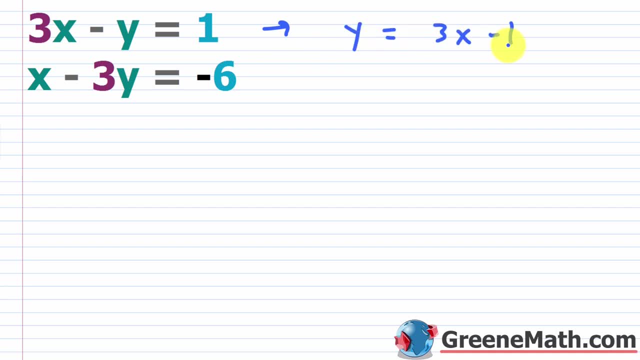 intercept form this is just going to be: y is equal to 3x minus 1.. Then for this one you would have negative. 3y is equal to. I'm going to subtract x away from each side, so I'll have minus x over. 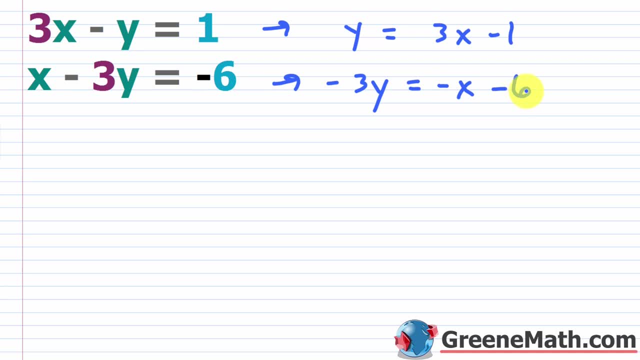 here and then minus 6.. I'm going to multiply both sides by negative 1- 3rd, so this would cancel. If I multiply this by negative 1- 3rd, this would be positive 1- 3rd and then negative 1- 3rd multiplied. 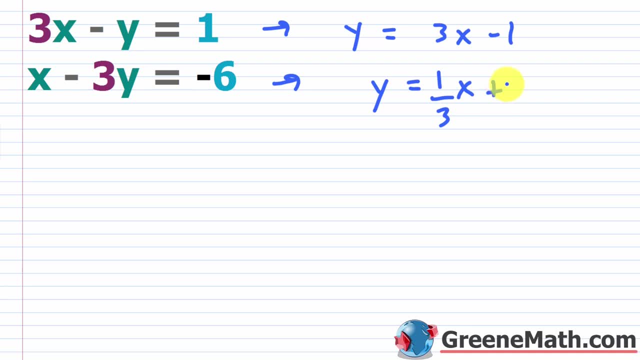 by x would be positive 6 divided by 3, which is positive 2,. okay, So this is my slope intercept form there. So if you wanted to graph these two, this one has a y-intercept of 0 comma, negative 1. 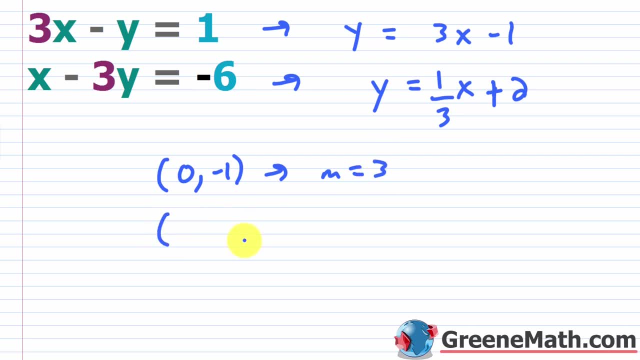 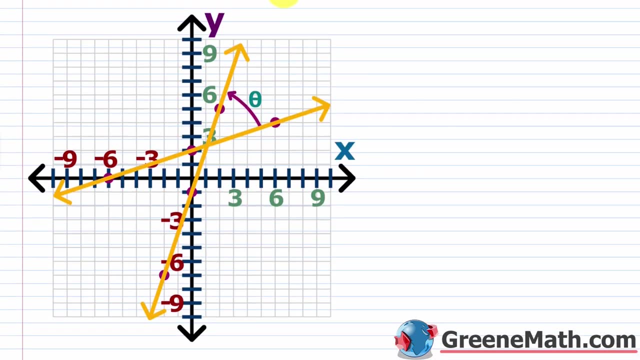 and a slope of 3, and then this one has a y-intercept of 0 comma 2 and a slope of 1. 3rd, Let me grab this real quick. Let's look at a graph real quick. Let me paste these in: 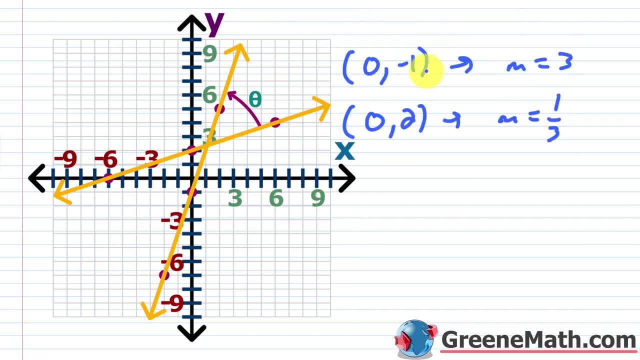 so we have some reference for where this stuff came from. So we have 0 comma negative 1, so basically right here, And the slope for this one is 3, so up 1, 2, 3 to the right 1, okay, So there's a point there. 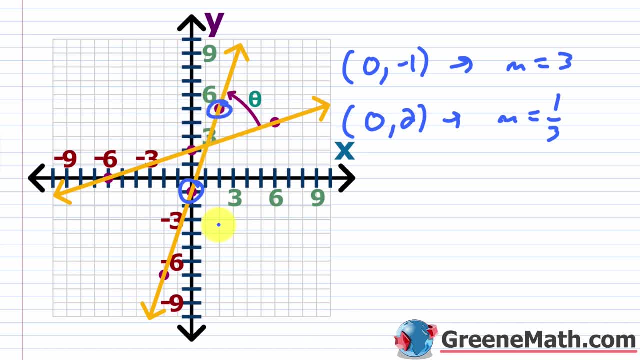 Then up 1,, 2,, 3 to the right 1, so there's another point there. okay, So that's this line right here, with a slope of 3, okay, Then the other guy is going to be 0 comma 2, so we have this guy, right. 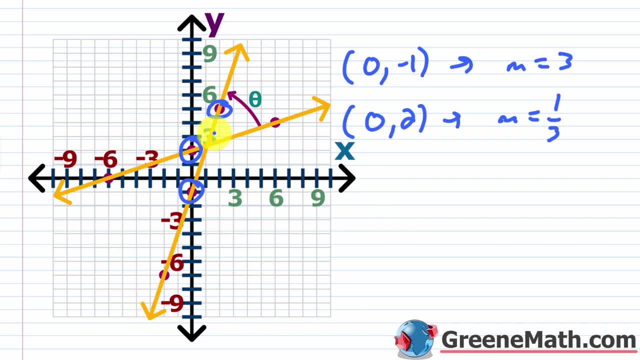 here. okay, The slope is 1, 3rd. so up 1 to the right- 1,, 2,, 3, so there's a point. Up 1 to the right- 1,, 2,, 3, so there's a point right there, okay. So you see how we get the graphs of these guys. 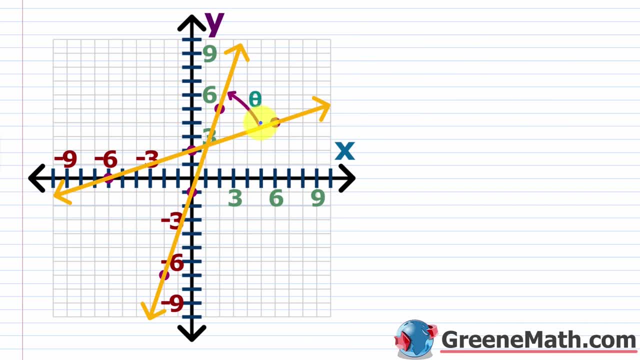 and what's important is to understand what you're looking for. You're looking for this angle right here, this acute angle, theta- okay. Now, in some cases you're going to want to find this angle right here and basically, once you've found this angle right here, you can subtract 180 degrees. 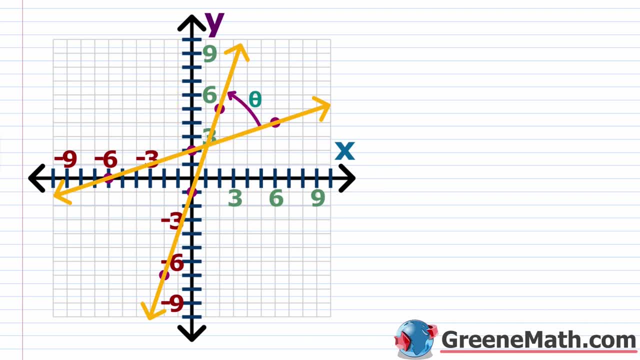 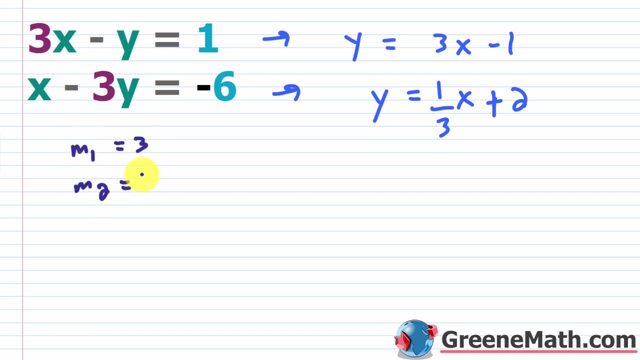 minus that angle, It'll give you this angle right here. So let's go back and let's think about how we can find this. I'm going to say that m sub 1 is equal to 3.. I'm going to say m sub 2 is equal to. 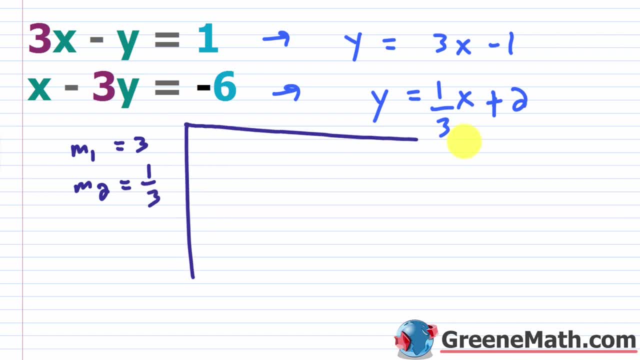 1, 3rd. and then I'm just going to plug into this angle right here and I'm going to find this angle to the formula that I had. So I'm going to say the tangent of theta is equal to, and remember: 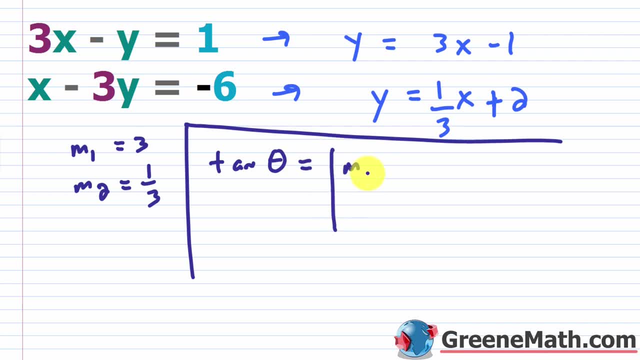 you're going to do m sub 2.. Actually I should probably write this out: So the absolute value of m sub 2 minus m sub 1, so that goes up here and then down here you're going to have 1 plus. 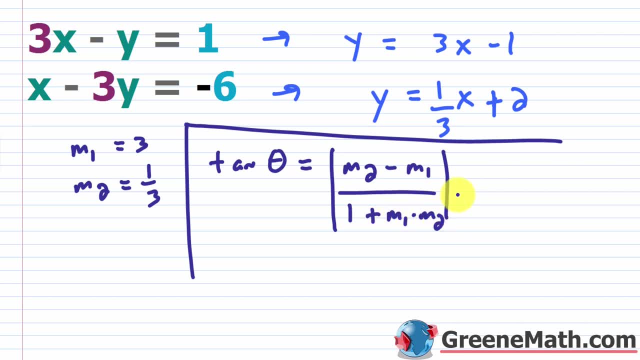 m sub 1 times m sub 2, okay. So my tangent of theta is going to be equal to- we're going to do the absolute value of. let's go ahead and do 1, 3rd, then minus 3, okay, And then down here. 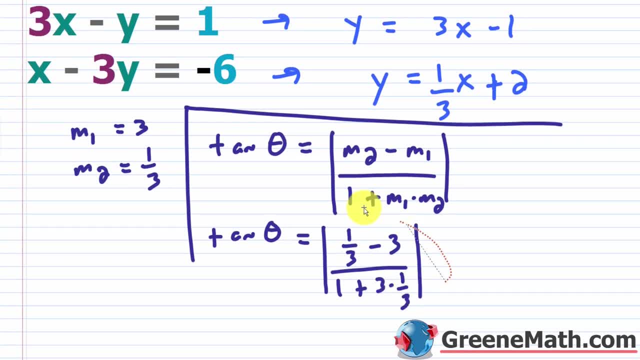 I'll do 1 plus you'll have 3 times 1 3rd. okay, Can't really fit this all on the screen, so let me cut this away. Let's go to this blank sheet here and see if we can just crank this out. 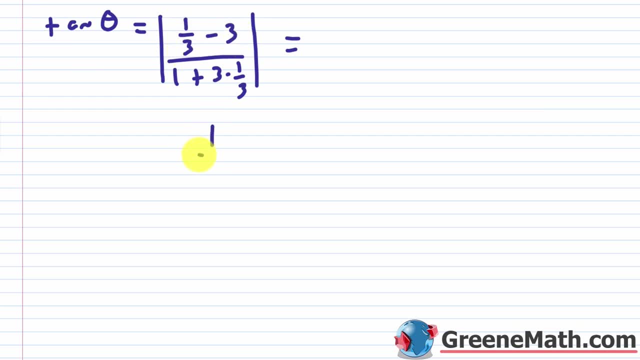 So this equals what? What is 1 3rd minus 3?? Well, you get a common denominator there. 3 would be 9, 3rds. Basically, 1 minus 9 is negative 8, so this would be negative 8, 3rds. Let me put my absolute. 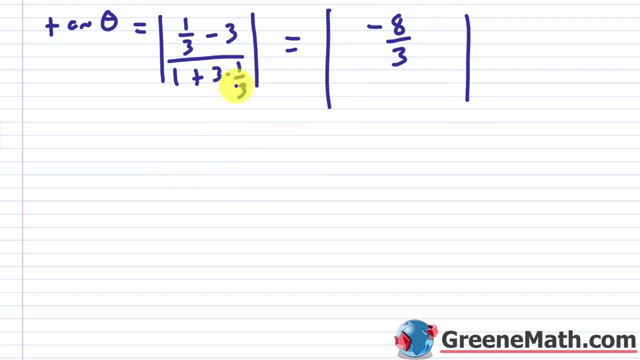 value bars in there, so don't forget them. And then basically down here: 3 times 1. 3rd is 1,, 1 plus 1 is 2, so this is divided by 2.. And then what I could do here is say: okay, this is the absolute value of negative 8 3rds. 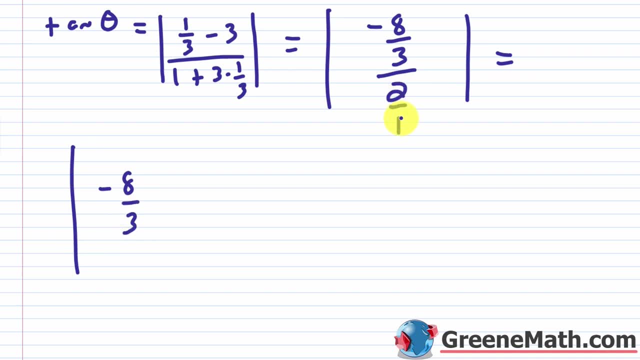 Since I'm dividing by 2, you can think about this as 2 over 1, just flip that guy, multiply, so times a half. okay, like this. So from here I can cancel this 8 with this 2 and get a 4 here. 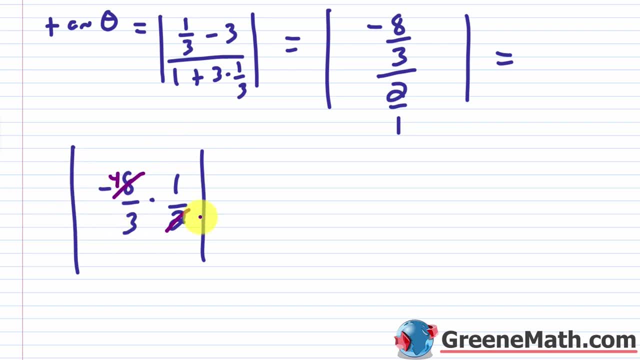 okay, So this would be negative 4 3rds, but we're taking the absolute value, so we end up with 4 3rds okay. That's important because, again, we want to get an acute angle. so when we do our 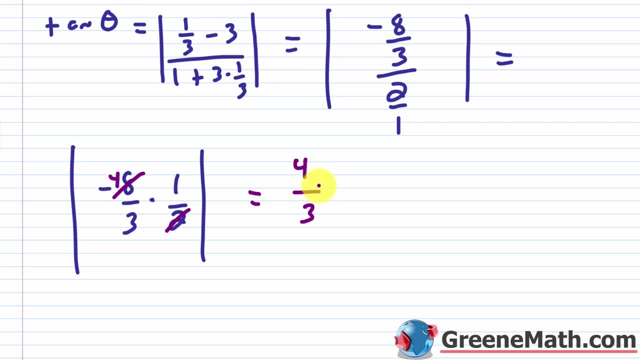 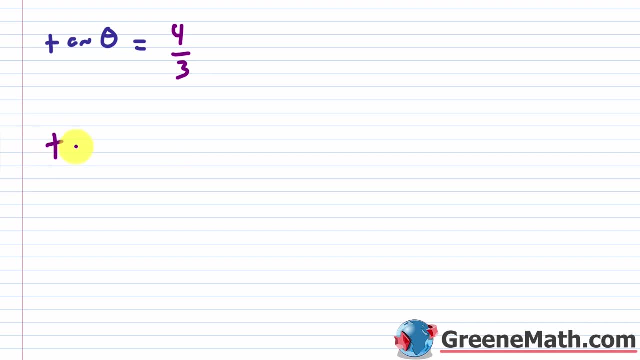 inverse tangent. we want this to be positive, so we get something in quadrant 1, okay, And let's bring this up here. So tangent of theta equals 4 3rds. What I'd want to do is say the inverse. 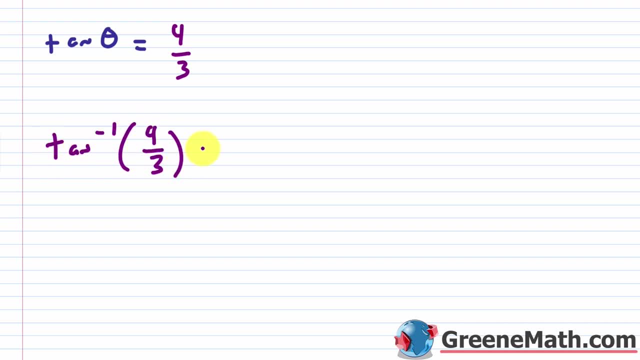 tangent. so the inverse tangent of 4 3rds is going to be equal to what? And I'll do an approximation here. I'll say this is about 53.13 degrees. Now, if you wanted the other angle again, 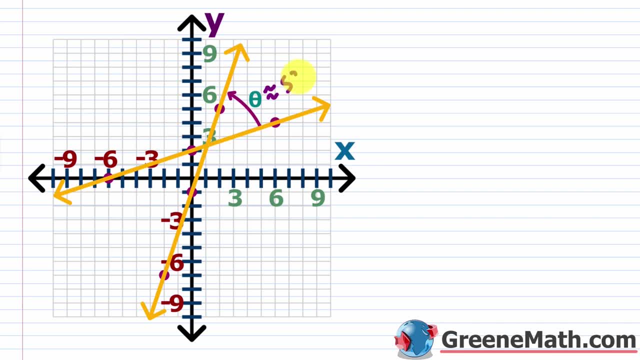 if you go back. this one is about: let me write this in 53.13 degrees Again, because this right here, okay. this angle right here would be a straight angle. all you'd have to do is take 180 degrees minus this angle here if you wanted this angle right here, okay. So if you wanted this, 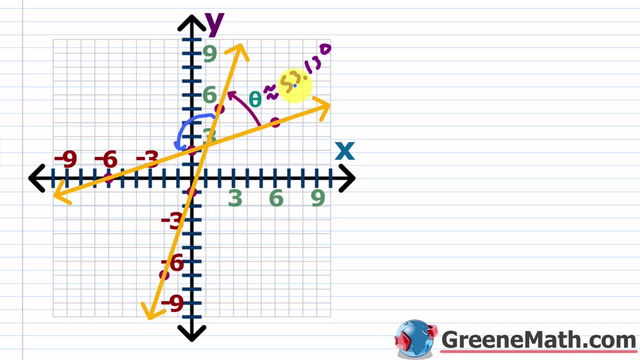 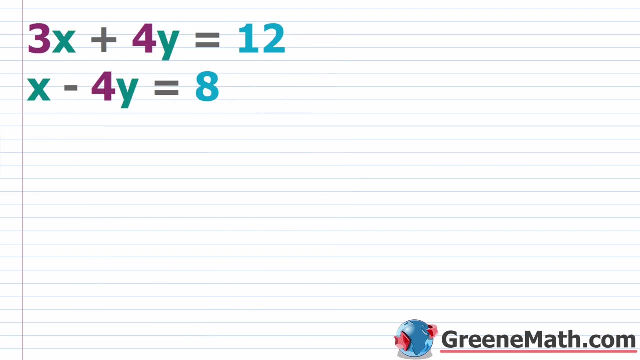 guy right here. you would say: 180 degrees minus 53.13 degrees. That would give you 126.87 approximately degrees. okay, So sometimes they'll ask you to get this one. Usually you're asked to find this one, but that's how you find both. Okay, pretty easy overall. Let's go ahead and take a. 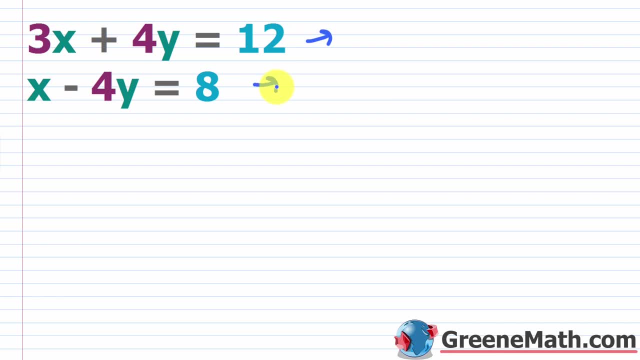 look at another example. So for this one again, I'm just going to put these in slope-intercept here. So I would say this is, 4y is equal to, I'm going to subtract 3x away from each side. 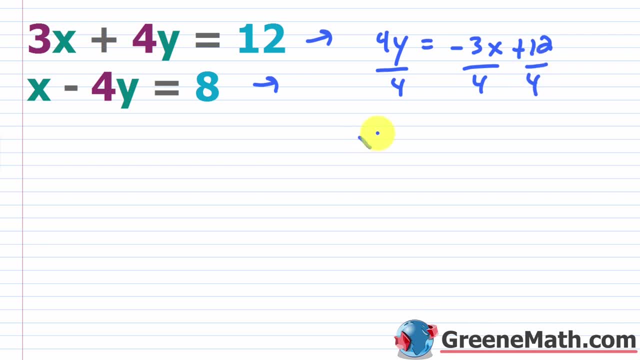 and I'm going to divide everything by 4.. So that would give me y is equal to: I'll have negative 3 4ths times x plus 3.. So my slope here, my m- let's call it m- sub 1, is equal to negative 3 4ths. 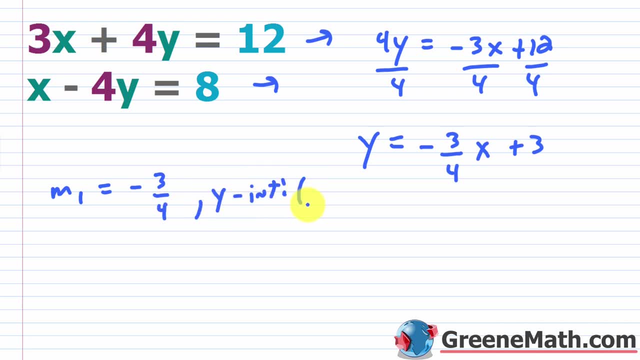 And I'm going to write the y-intercept just so we can graph it and see what it looks like. Again, not necessary. So this is 0,3.. Just doing it to get a full view of what's going on. So let's. 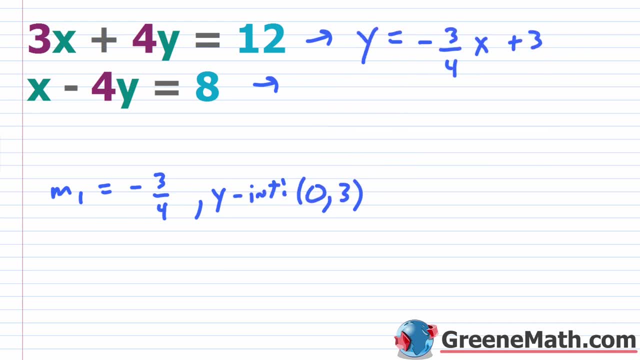 and let's drag this up here. okay, Let me change my ink color For this one. I would do what Negative 4y is equal to subtract x away from each side. so negative x plus 8. Divide everything by. 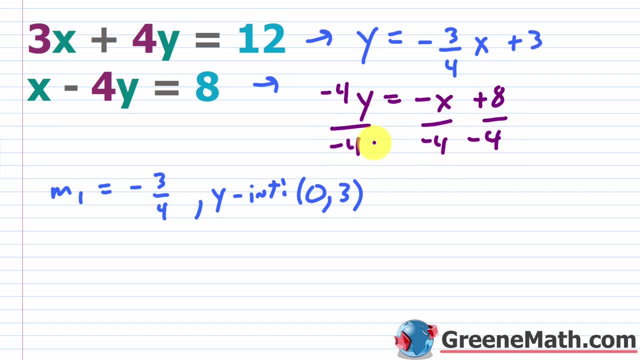 negative 4,. okay, And that's going to give me that y is equal to 1 4th x. So let's put this as 1 4th x And this would be minus 2, right, So minus 2.. So m sub 2, let's say this is 1 4th here. 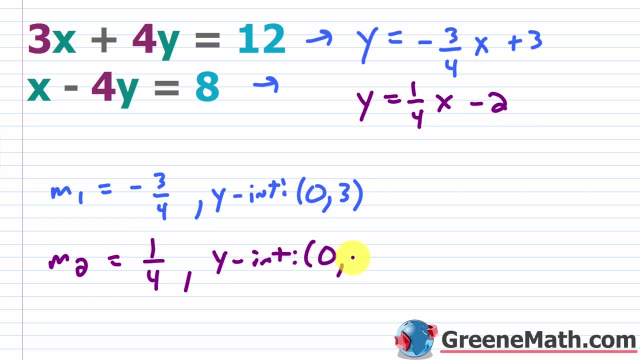 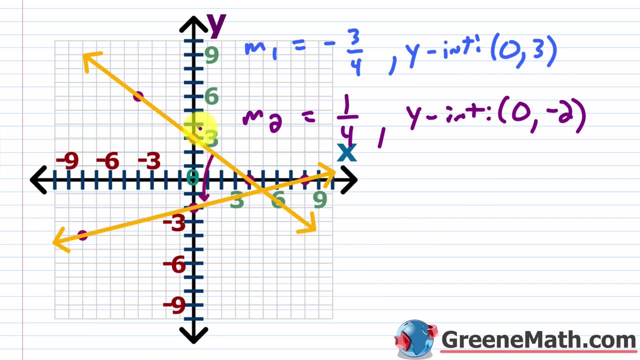 And my y-intercept is going to occur at 0 comma negative 2.. Again, let's copy this real quick. Let's look at the graph. So the y-intercept is at 0 comma 3, so it's going to be right there. And then the slope is. 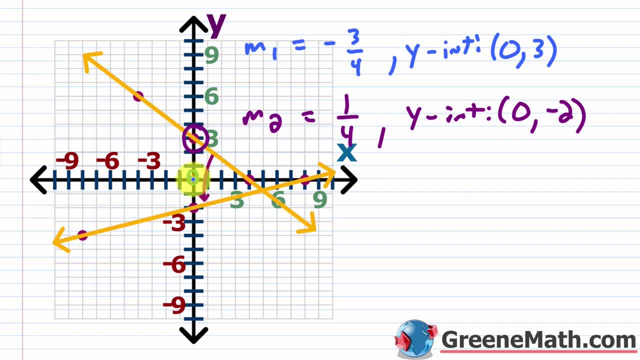 negative 3, 4ths. So down 1, 2, 3, to the right: 1,, 2,, 3, 4.. So that's that point right there. Then the other guy is 0 comma negative 2, so just drop by 2, so it's right there. And then basically, 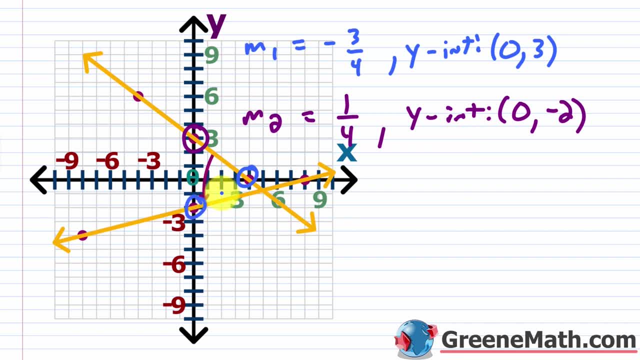 the slope is 1, 4th, So I can go up 1 to the right- 1,, 2,, 3, 4.. Okay, there's a point. Then up 1 to the left: 1,, 2,, 3, 4.. There's a point. Okay, so we see where these graphs came from. And again, 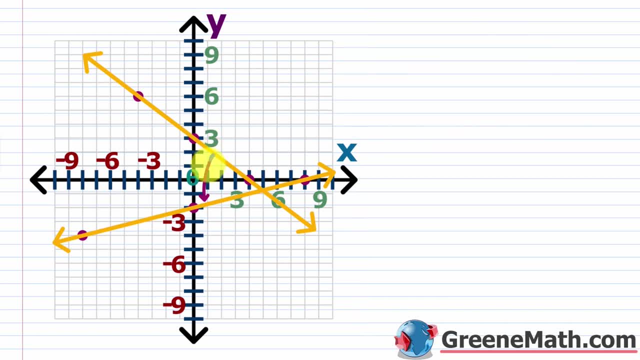 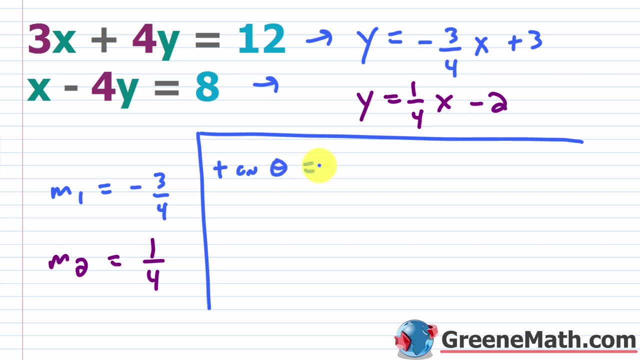 what are we trying to figure out? We're trying to figure out what is this angle right here And I'm just going to plug into my formula, So let me box this off. So the tangent of theta again. hopefully you have this written down. It's the absolute value of you're going to do m sub 2,. 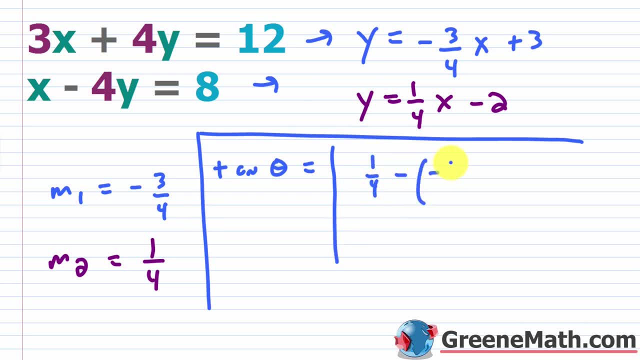 which is a 4th minus m sub 1, which is negative 3 4ths, And I'll just leave that like that for now. I'll just simplify as I go. Then it's going to be 1 plus the product, which is negative 3 4ths. 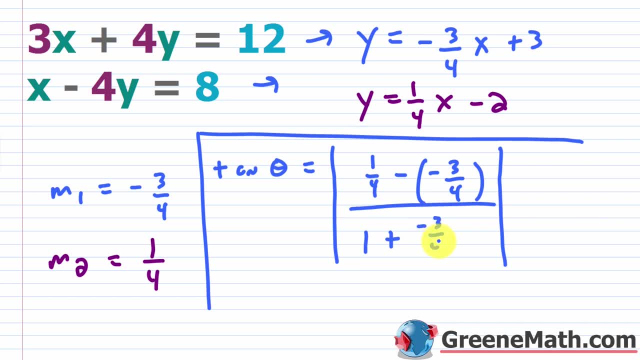 So you'll have your negative 3 4ths and then times your 1 4th. Okay, so 1 4th minus a negative 3 4ths is like 1 4th plus 3 4ths. There's already a common denominator, so it's just 1 plus 3,. 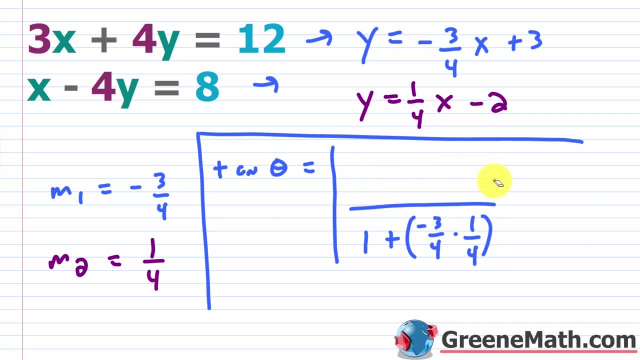 which is 4, over 4, which is basically just going to give us 1.. Okay, so that part is very simple Down here. if you multiply these together you would end up with negative 3 16ths. So this down here is minus 3 16ths. 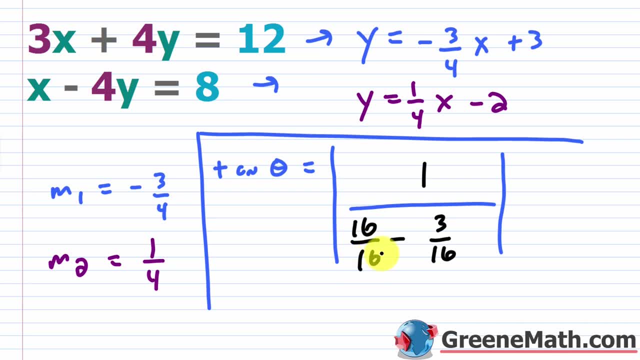 The 1 there can be written as 16 over 16.. And, of course, if you subtract you would get 13 over 16.. So 13 over 16.. Now this is already positive, so you can go ahead and drop the absolute value bars. 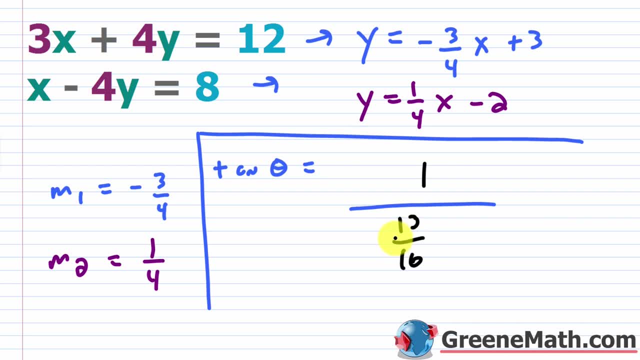 You don't need them. And then, basically, if I take 1 and divide by this fraction, all I need to do is flip the fraction right. So essentially this ends up being 16 over 13.. So 16 over 13.. So let's punch up in our calculator tangent inverse of 16 over 13 and see what we get. 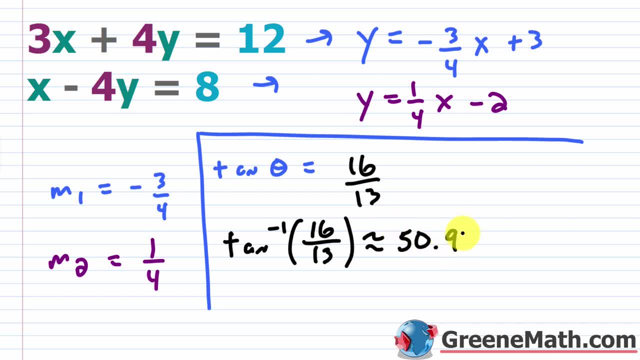 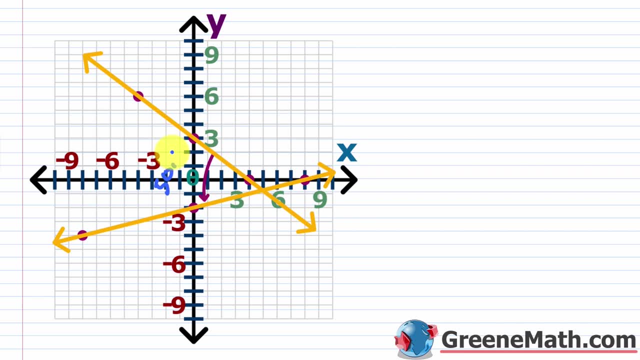 So we've got about 50 point. I'll go ahead and say 9, 1 degrees. So if we go back, so this angle, theta is about 50 point and I'll say 9, 1 degrees Again, if you're looking for this angle here, okay, remember this guy right here. 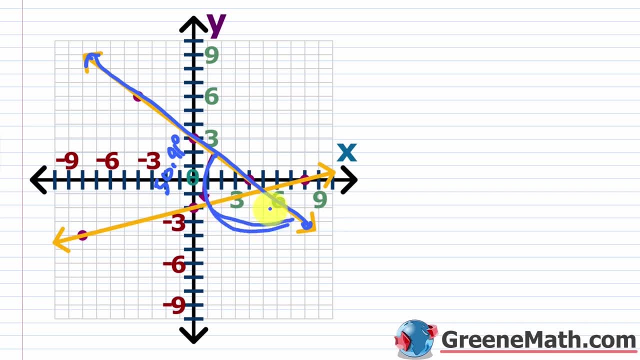 if you consider this as a straight line, right? so this whole thing is 180 degrees. I know we're flipped upside down so it's a little bit hard to see, But this angle right here, if you think about it, would just be 180 degrees. 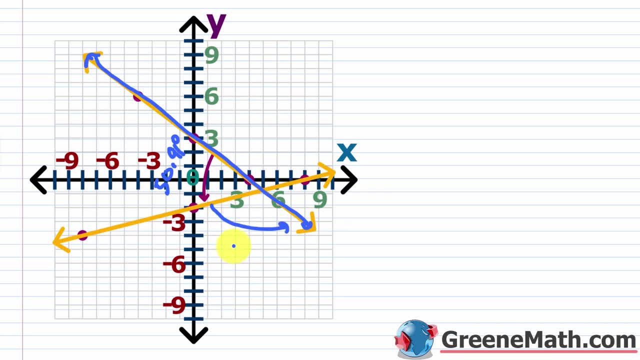 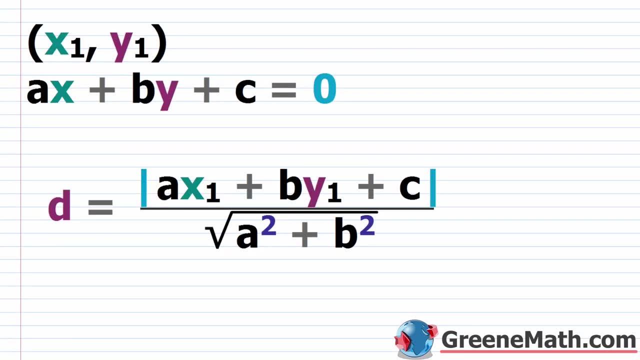 minus 50.91 degrees, So it will be about 129.09 degrees. if you need that angle, All right. so the last concept we're going to talk about is how to find the shortest distance from some line that you're given to a point that is not on the line. Okay, 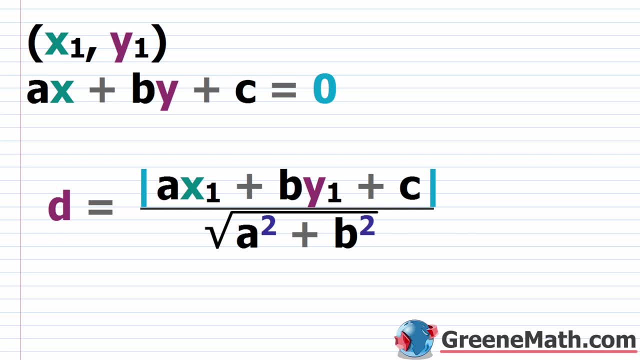 so what I'm going to do here is give you a simple formula that you can plug into. Instead of going through and deriving this specific formula, I'll show you how you can go through a similar thought process, And I'm going to go through a similar thought process. 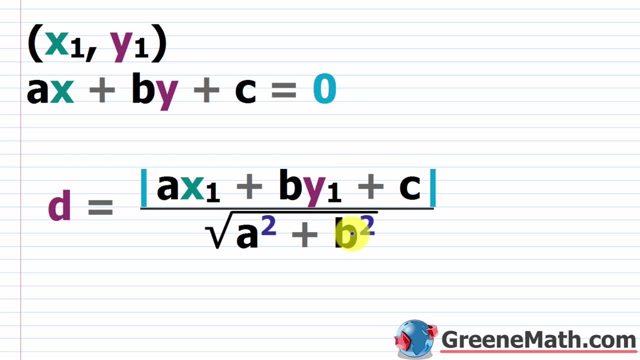 and I'm going to go through a similar thought process. and I'm going to go through a similar thought process with our actual example. Okay, I think it's a little bit easier to comprehend. So let's say that we start with some point: x sub 1 comma, y sub 1.. Okay, and it's not on this line. 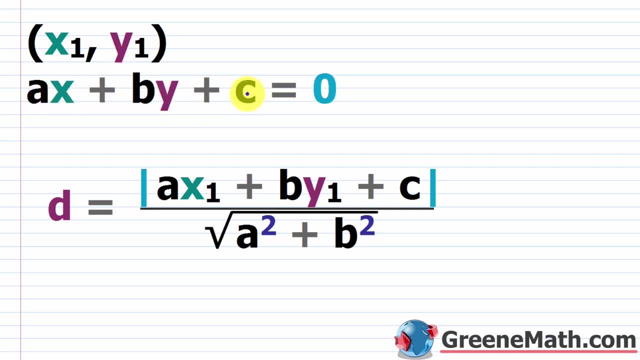 that we're given, which has the format of ax plus by plus c equals zero. Okay, if you want the shortest distance from this point to this line, then you can plug in to our little formula here where we say d, the distance is equal to. you have absolute value. bars on the top. 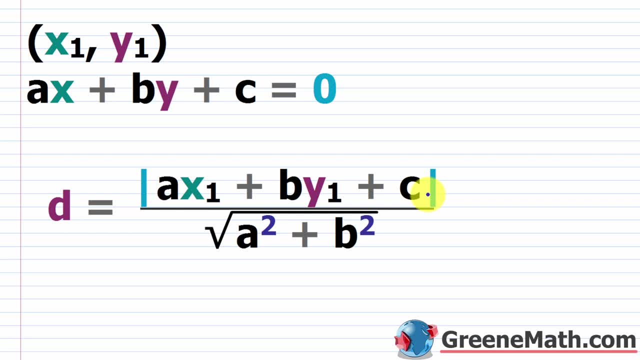 you're going to need them to make sure that you get a result that's going to be positive. you can notice that your a, your b and your c here are coming from your equation of the law. right? Here's your a. it's the coefficient for x. here's your b. 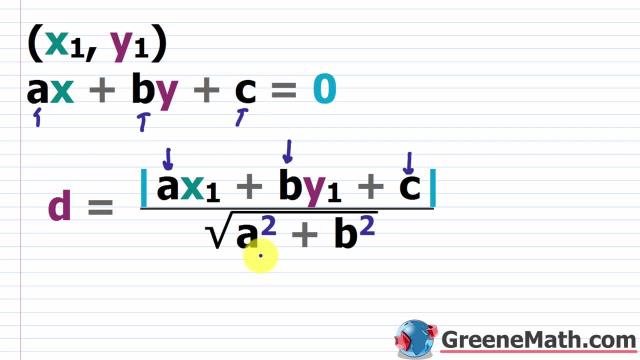 it's the coefficient for y, and here's your c, it's your constant. Okay, then, when you see that down here, it's the same thing. Okay, Now, when we talk about the x sub 1 and the y sub 1, this: 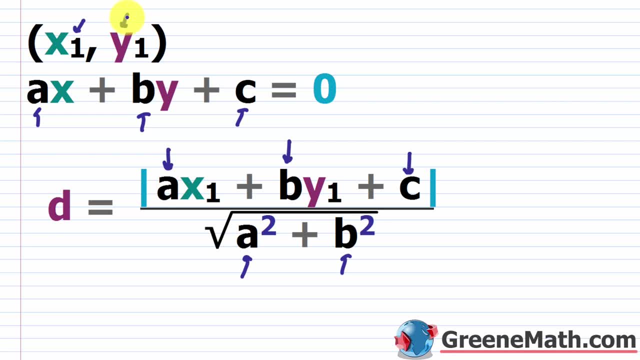 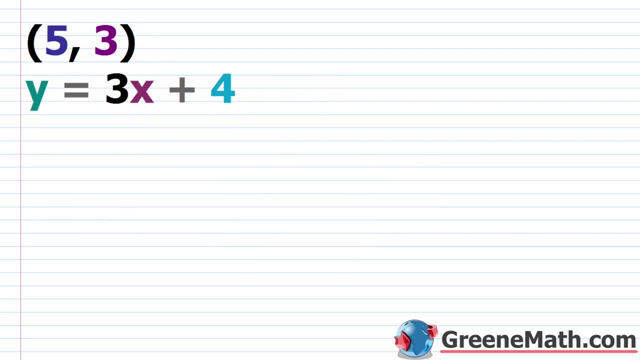 is coming from your point that you're given: Okay. So let's just try this out really quickly on an example And then I'll show you where this comes from. So let's say, we're given the point five comma three and we're given the line y equals three x. 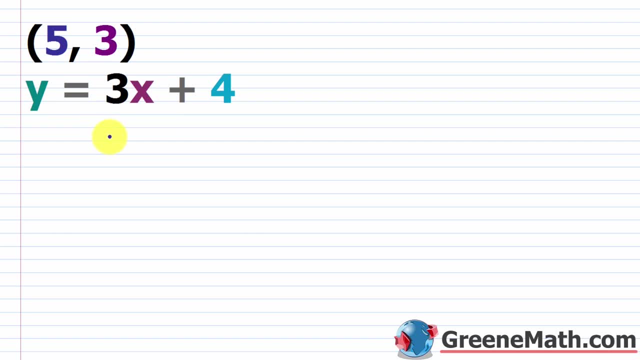 plus four. Okay, The first thing is you want to rewrite this. you have to have this in the form of ax plus by, and then plus c is equal to zero. Okay, people often make the mistake of writing this as ax plus by equals c. Okay, that's what you're used to for standard form, But we need 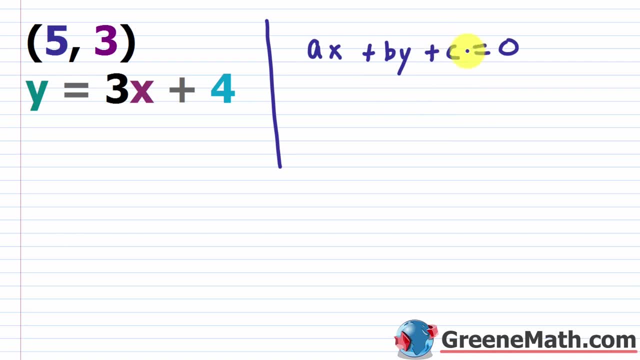 to put it into this form in order for that formula to work. Okay, So what I'm going to do is I'm going to subtract y away from each side of the equation, And so that would give me. let me line this up. 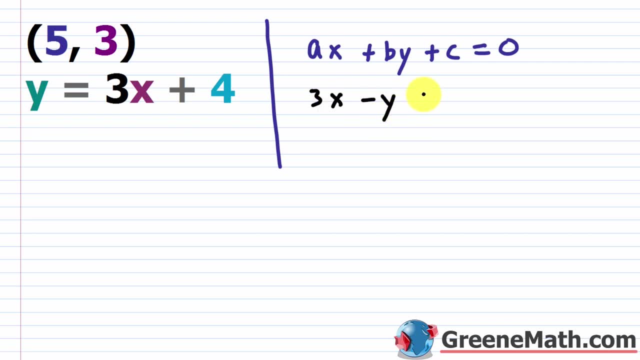 three x, and I would have minus y, and then I would have plus four and this equals zero. Okay, So if you want to line things up here, you would say a is three, So a is equal to three, then b is equal to what You have- a negative y. I could put a negative one there to make that clear. 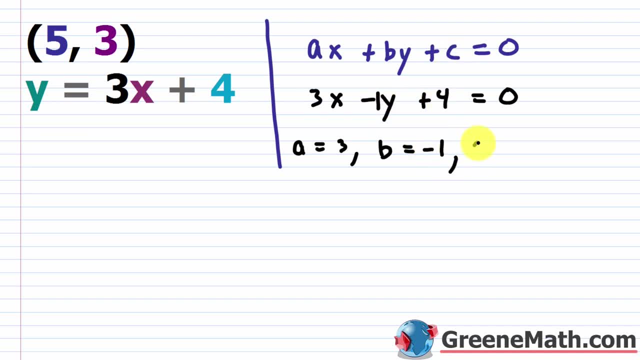 that the coefficient is negative one, and then c, your constant term is going to be four. Okay, Then when we talk about the x sub one, it's the x coordinate from the point. so that's five. And then your y sub one is the y coordinate. 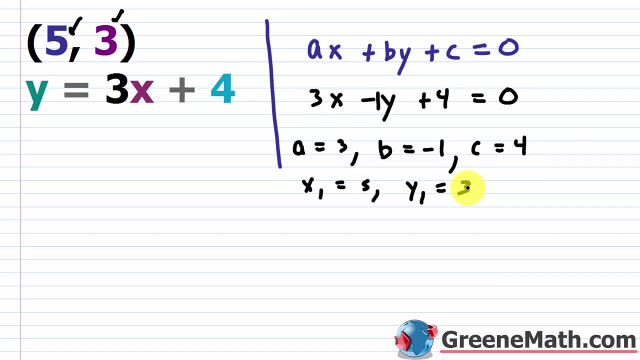 from the point. so that's three. Okay, So this is all you really need to do: just figure out how you can put this into this format and just grab the values that you need. So now I'm just going to plug into the formula. So my distance is equal, to remember, you want. 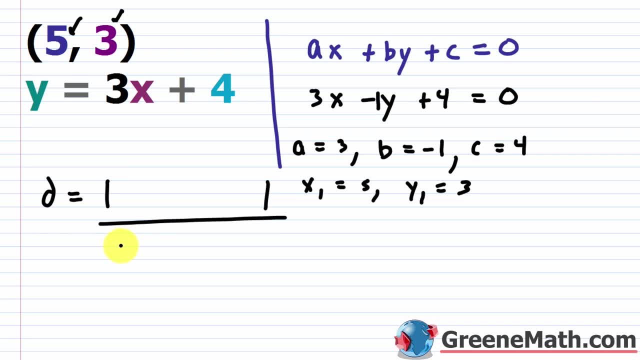 the absolute value bars. And then when we put this over, the bottom part's easy. So square root of a squared, so a squared plus b squared Up here, remember you would take your a times your x sub one plus your b times your y sub one. 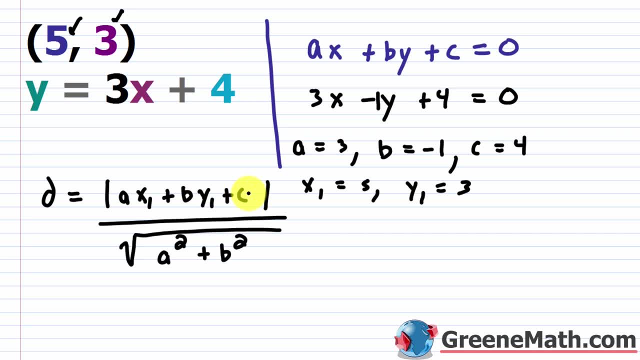 and then plus your c. Okay. So that's a pretty easy thing to remember after you do it a few times. Let me go ahead and see if I can move this up, And let's go ahead and paste that right there. Let's erase that, make this border a little bit better, Okay. So if we plug in here, we'll have 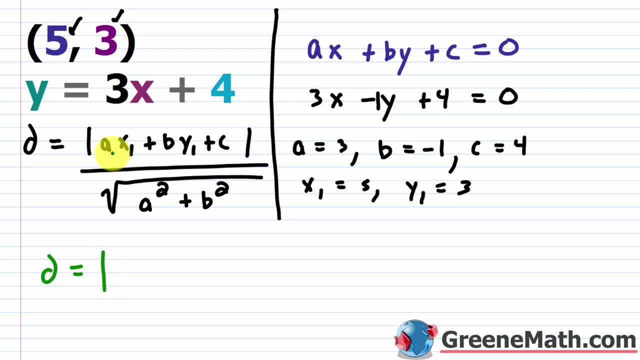 d is equal to the absolute value of. we have a, which is three. let me write this out: So, three times your x sub one, which is five, And then plus your b, which is negative, one times you're going to have your y sub one. 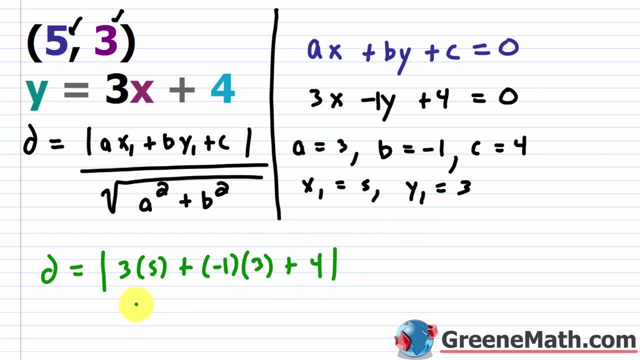 which is three, And then plus your c, which is four. Okay, close that down And this is over the square root of. you'd have a squared, so three squared, plus b squared, So negative one. wrap that, in parentheses, squared. Okay, Let's go down and get a little bit of room going so we can. 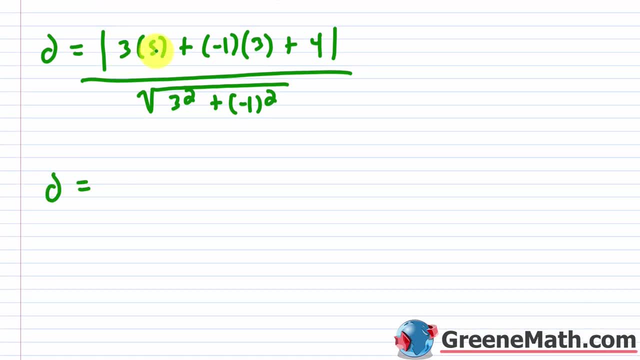 work on this. So d is equal to three times five is 15.. So let me write this: 15.. Negative one times three is negative three. So negative one times three is negative three. So negative one times minus three, And then we'd have plus four. Okay, So if we do 15 minus three, that's 12.. And then 12. 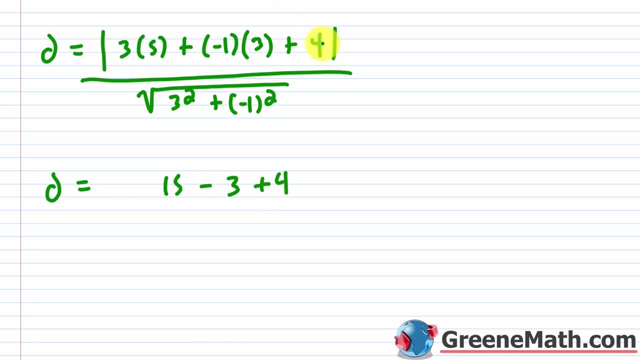 plus four is going to give me 16.. Okay, So you have the absolute value bar. you can wrap it in that, But this is going to be positive, So you really don't need them in this case. This is basically just going to give you positive 16 up here. Okay, Then in the denominator you have three. 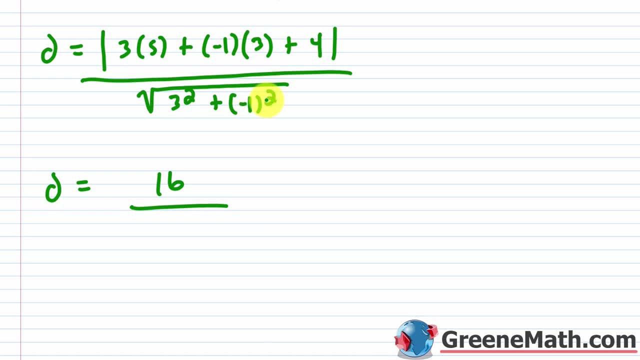 squared, which is nine, and you have negative one squared, which is one. So nine plus one is 10.. So this is the square root of 10.. Okay, Now we know that we don't leave the radicals in the denominator, So let me fix this by multiplying the numerator. 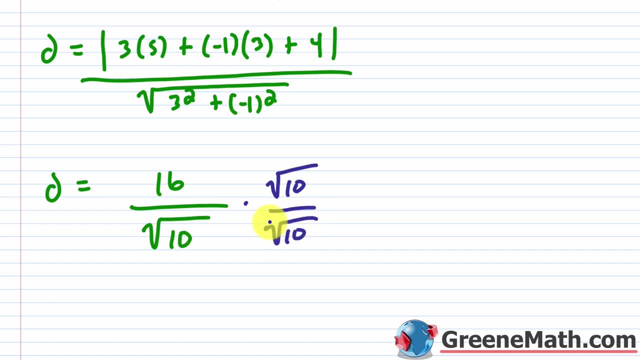 and the denominator by the square root of 10, right. So what we'd have here is that you'd have 16 times the square root of 10 over square root of 10. times square root of 10 is 10.. Now you can simplify this further, because, between the numerator and denominator, 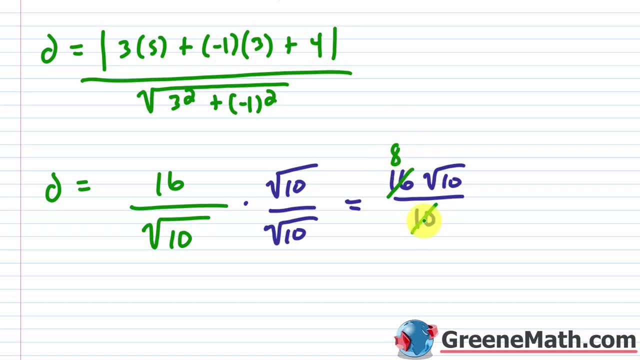 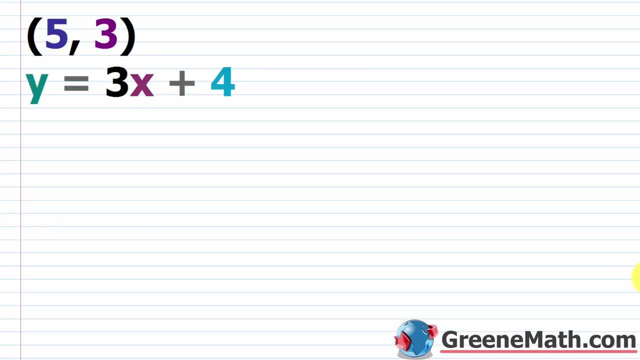 we have a common factor of two. So this, divided by two, is eight. this divided by two is five. So the final answer is going to be eight times the square root of 10 over five. Okay, So now let me give you a little bit of insight. 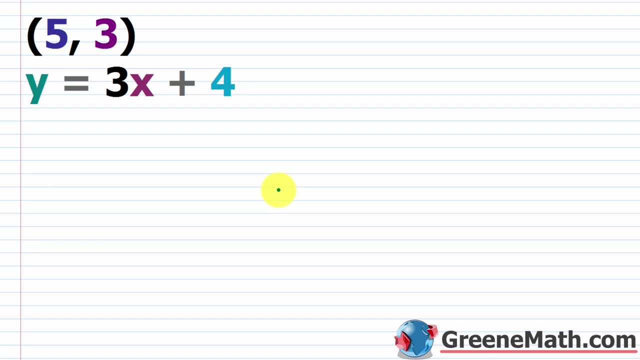 Into where this formula comes from. I'm not going to use the generic notation because every time I teach that I find that students get lost. So using an actual example is a little bit easier to comprehend. So the first thing is I want to think about if I want the shortest distance. 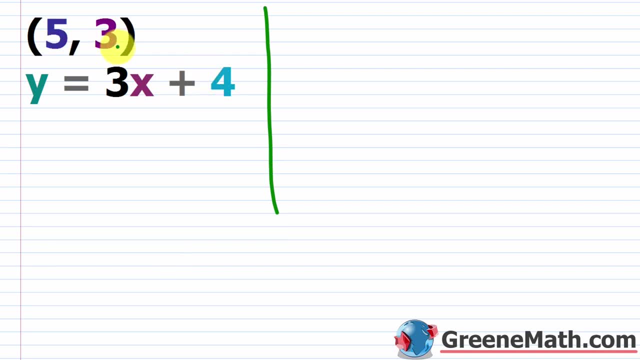 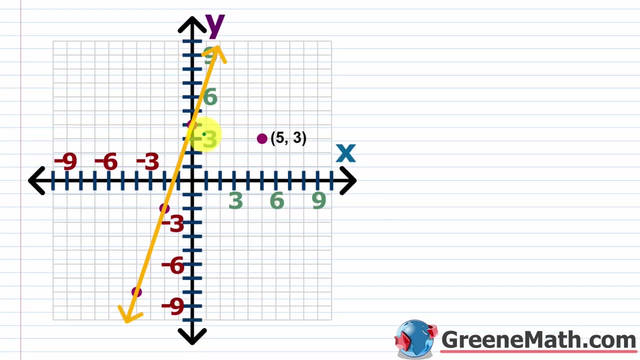 between this line and this point, which is not on the line. what's going to happen is: I'm going to need to find- let me go to a little image here- I'm going to need to find the perpendicular line segment That's going to join this point here and this line. 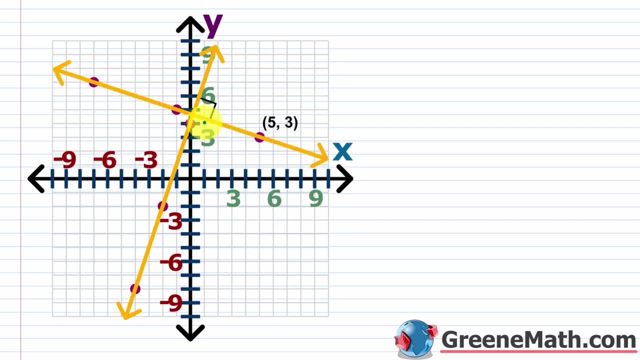 Okay, So what you could draw is a little line like this: Okay, And I'll show you how to get this line in a moment, but basically you're looking for the distance from this point to this point, right here. Okay, If you just took this part of the line. okay, that's the line segment that. 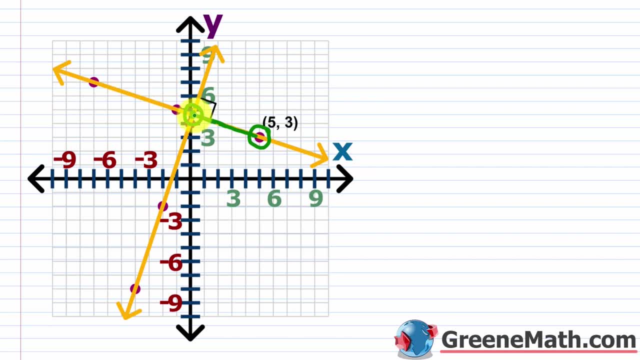 connects this point right here, which is the point of intersection, Okay, And this point right here, which is five comma three. that is the shortest distance from this point to this line. Okay, You can see we have a little right angle that's formed, because these guys are going to be. 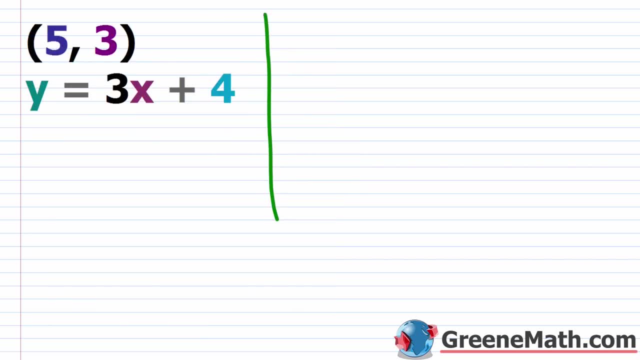 perpendicular. So let's go back. Having viewed this, let's think about a few things. First and foremost, perpendicular lines have slopes whose product is negative one. So if the slope here is three, so if my first slope, M, is three, let's call this M sub one, then M sub two would have to be. 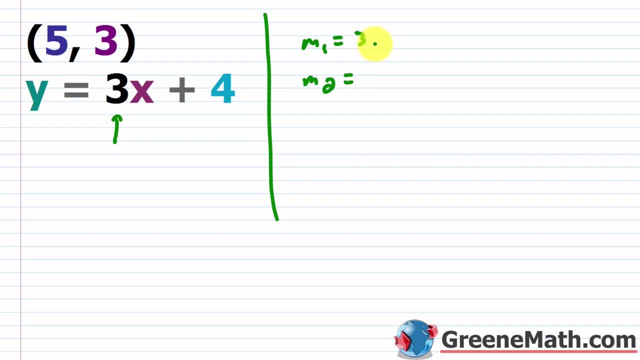 what we can go through and set up an equation for that, but you really don't need it. Three times what would give me negative one. three times negative one. third, right, It's always the negative reciprocal of the number, right? So flip the number, you get one. 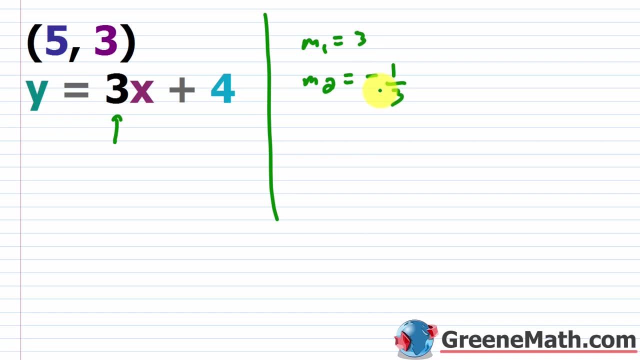 third, take the negative of it. you get negative one third. Okay, So now what I can do is I can say: okay, well, I know my slope. Let me just get rid of this. I'll just say I know my slope over here. 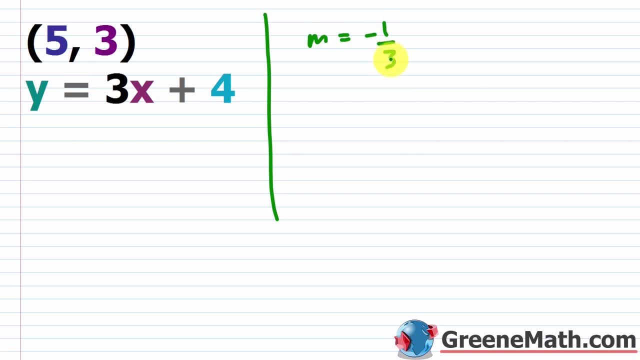 my M is negative one third. but how do I get the equation of the line? Remember, I know this point right here is on the line. So if I have a point and I have the slope, then I can use point slope formula. Okay, So I can say: Y minus Y sub one is equal to M times the quantity X minus X sub one. 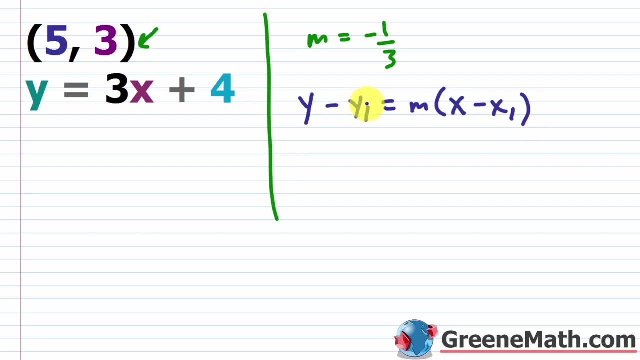 I know it's been a while since we used that, but basically I would plug in for X sub one and Y sub one. So my X sub one is five. Let's plug that in. My Y sub one is going to be three. plug that in. 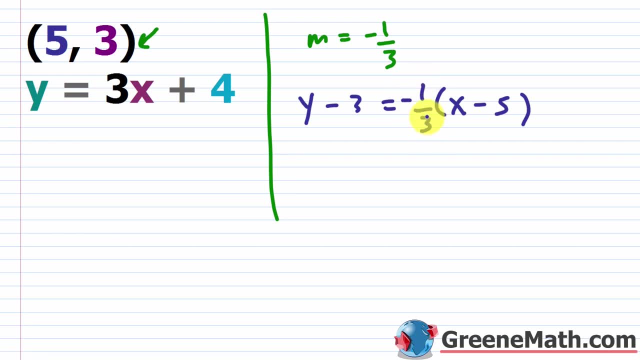 And my M. my slope is negative one third, So negative one third. Okay, So we can get rid of this And basically from here I can distribute this. Let's say Y minus three is equal to negative one third. X, and then plus five thirds. You could solve for Y by adding three to both. 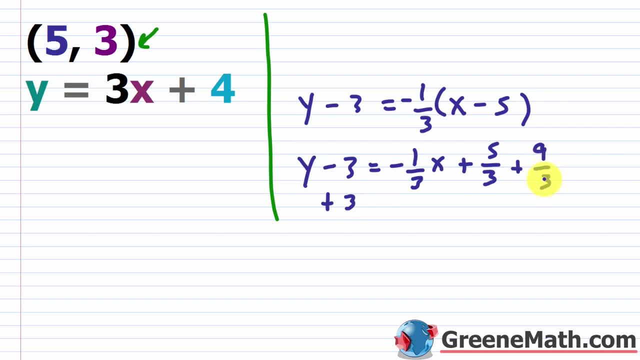 sides of the equation. Let's call this nine thirds, So we can have a common denominator. Let's get rid of this from over here. So I'll put: Y is equal to negative one third. X plus this will be 14 thirds. Okay, So this will be 14 thirds. So let's come over here and say Y. 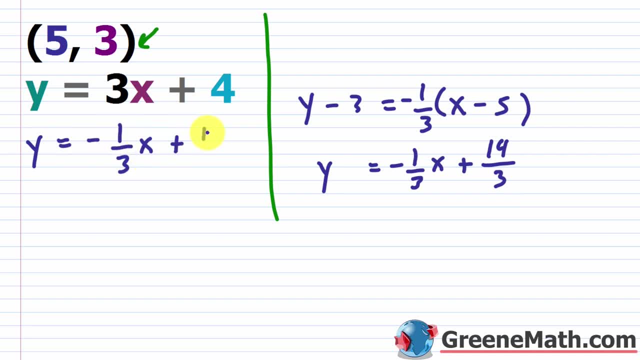 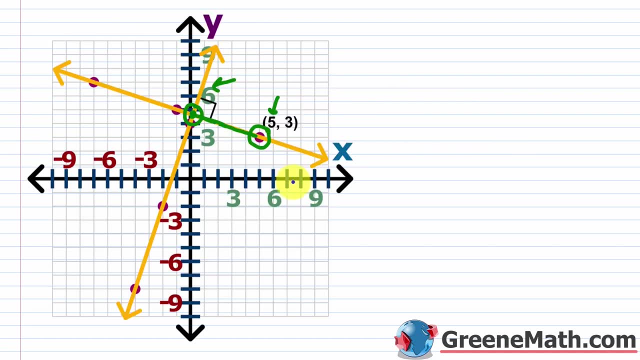 is equal to negative one third, X, and then plus 14 thirds. Okay, So now that we have that done, if we go back to the two graphs, you can see that the slope of this line is negative one third. If I started, let me erase all this kind of marked it up. If I started, let's say right here: 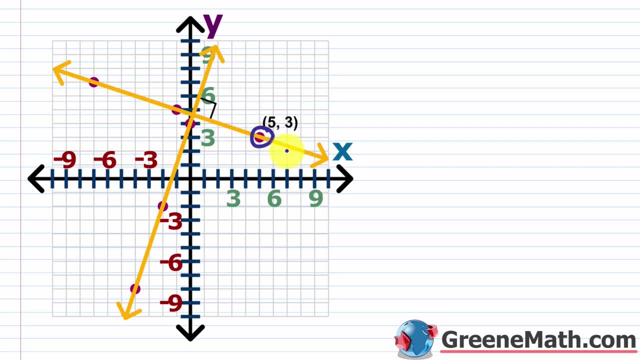 okay, which is a point on the line. If I drop one and I go to the right one, two, three, I'm back on the line. Okay, So you can see. that's where the slope is. The Y intercept is unfortunately not an integer value, but you could check other points on the line to make sure you. 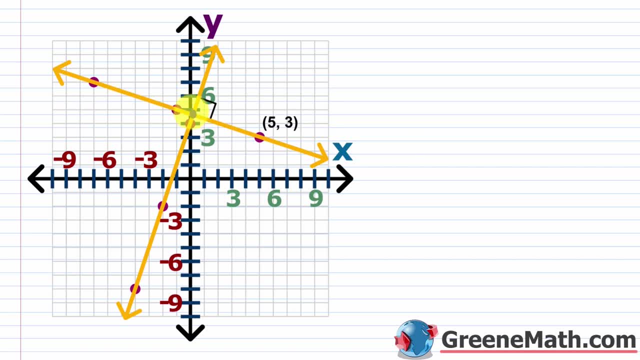 got it correct. Now, how can we find this point right here, the point of intersection? Remember, this is nothing more than just solving a system of linear equations- right, We're trying to find the point that basically satisfies both. So if we go back and we think 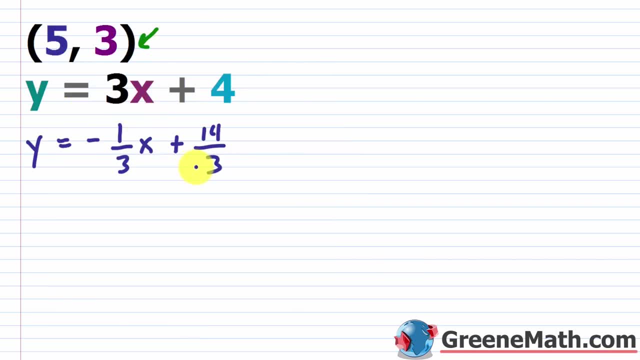 about this. we have each one solved for Y, So what I could do is I could actually set this guy right here equal to this guy right here, Y. I'm doing nothing more than just the substitution method. If Y is equal to this, well then I can just plug this in for Y, right there, right, That's all I'm. 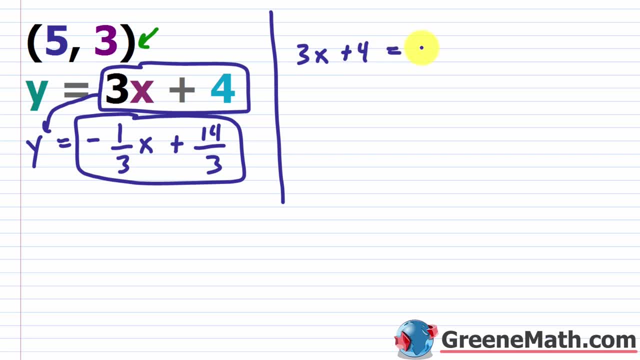 really doing So I could say three X plus four is equal to negative. one third times X plus 14 thirds. Okay, And then I just want to solve for X. figure out what that's going to be. So let's multiply everything by three. get rid of the denominators. This is nine. X plus 12 is equal to. 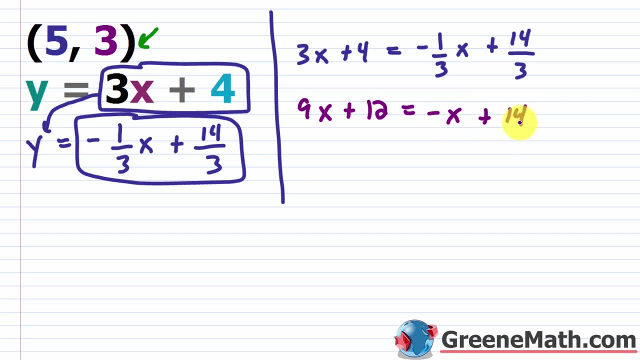 we'll put negative X and then plus 14.. Okay, So now it's going to make it a little bit easier. Let's go ahead and add X to both sides of the equation, Let's subtract 12 from both sides of the equation, And so this is going to cancel, and this is going to cancel. So you have 10. X is equal. 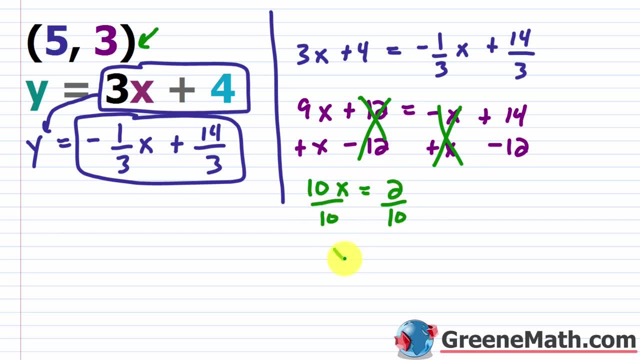 to. we'll say: two, divide both sides by 10.. You'll get: X is equal to one fifth. Okay, So the X value that we're looking for is a fifth. So let me put that in here. So the X value, X, is equal to one fifth. So the Y value is equal to. 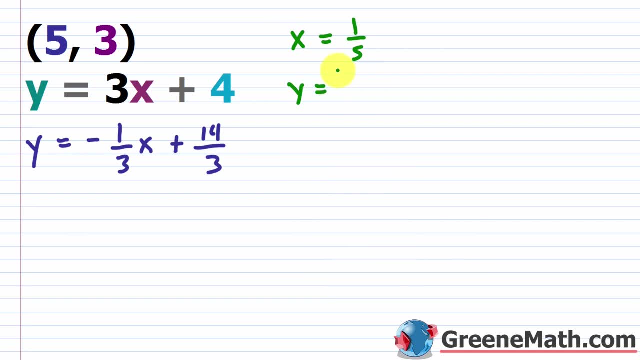 what Remember? if the X value is one fifth, it's one fifth here and it's also one fifth here. So I can plug it into either original equation and solve for the corresponding Y value. Again, this is going to be the point that solves both. Okay, So we'll go ahead and say Y is equal to. 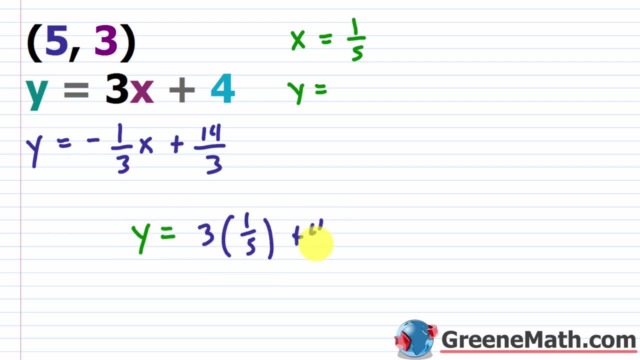 I'll say three times one fifth, and then plus four. Okay, So three times a fifth is going to be three fifths. So let's say this is three fifths. I need a common denominator, So let's write this as 20 fifths, right? 20 divided by five is four, So basically this is going to be 23 fifths. 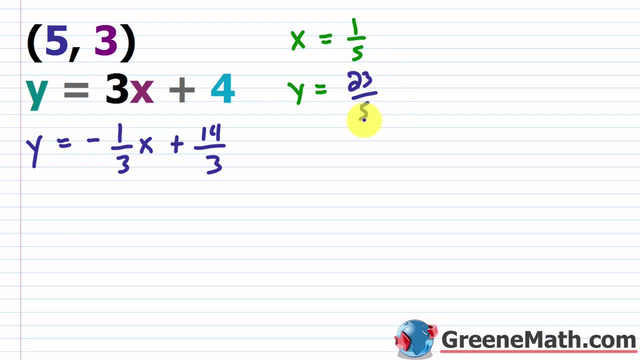 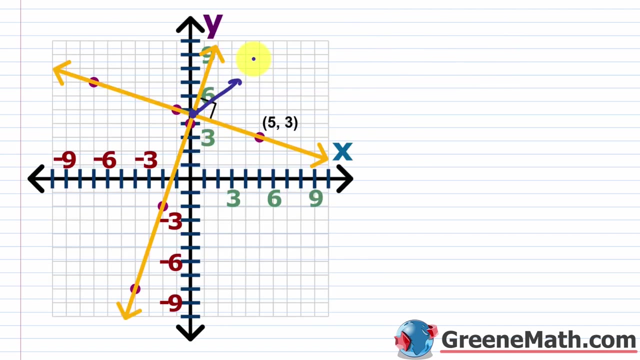 So Y is 23 fifths. Okay, So not the nicest point that you could come up with, but still you can work with it. So the point of intersection for these two lines is going to be comma 23 fifths, And if you go back, that looks about right. So we can say: this guy right here. 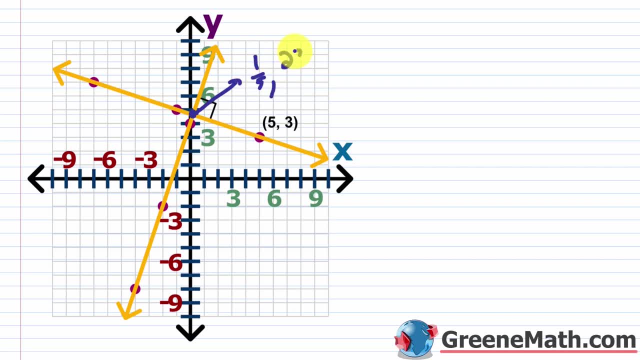 would be one fifth. Okay, That's the X coordinate, comma 23 fifths. That is your Y coordinate. Okay, So now I just need to find the distance between this point and this point here. Okay, That's all I want to do, And that's just the regular distance formula. So the distance is equal to remember the. 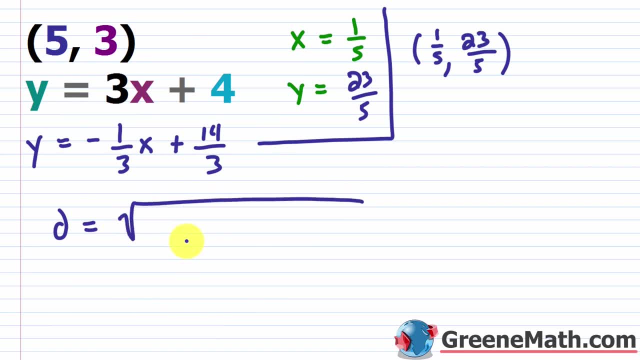 square root of you would take the difference in X values. So I can go ahead and say this is, let's say, my second point right here. So I'll say this is my X sub two comma, Y sub two, And remember we're working with. 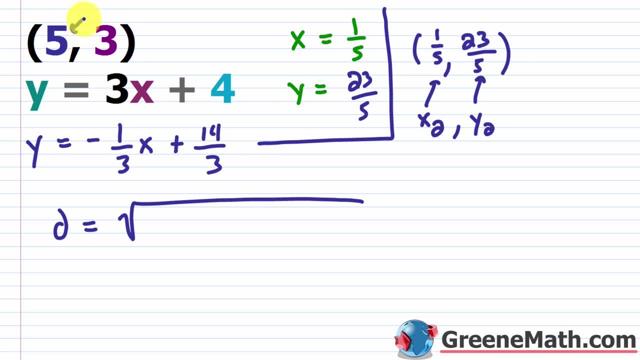 this point right here, because this is the point we're trying to find the distance to. So we'll say this is X sub one. We'll say this is Y sub one. Okay, So you want your X sub two minus your X sub one. So one fifth minus your five. this is going to be squared Plus you're. 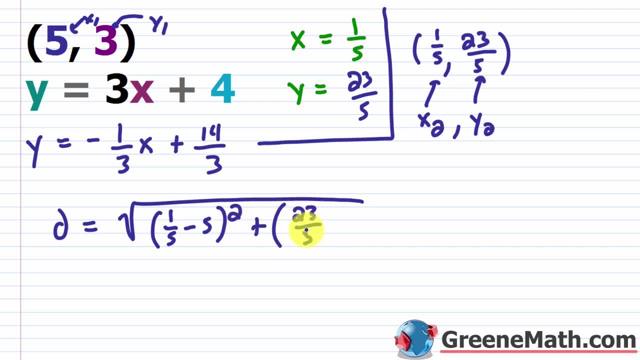 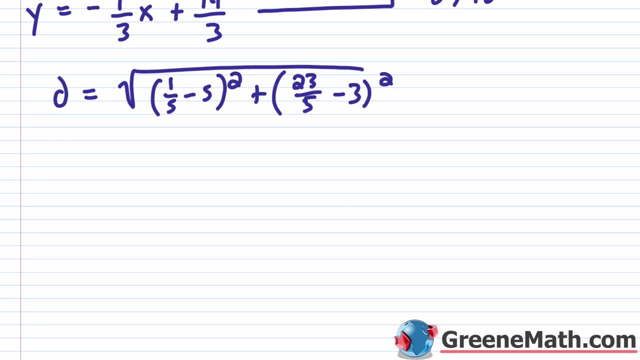 going to take your 23 fifths, So your 23 fifths, and this is going to be minus three, And then this is going to be squared, Okay. So I know a lot of you don't like working with fractions, but it's really not that bad. So the distance is equal to the square root of, so I need a common 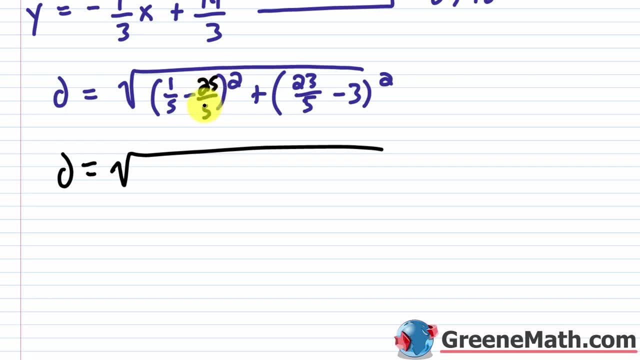 denominator here. Let's write this as 25 fifths. And let's go ahead and write this as 15, 15 over five. Okay, So one minus 25 is going to be negative 24.. So this is negative 24 fifths. This is going. 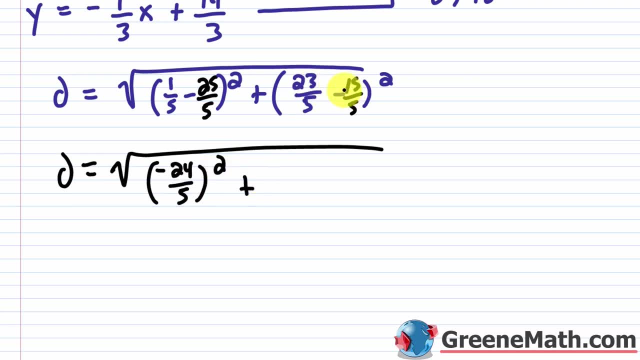 to be squared. Then plus 23 minus 15 is going to give me eight. So this would be eight fifths And this is going to be squared. Okay, So the distance is equal to the square root of. if you square five, obviously you get 25.. 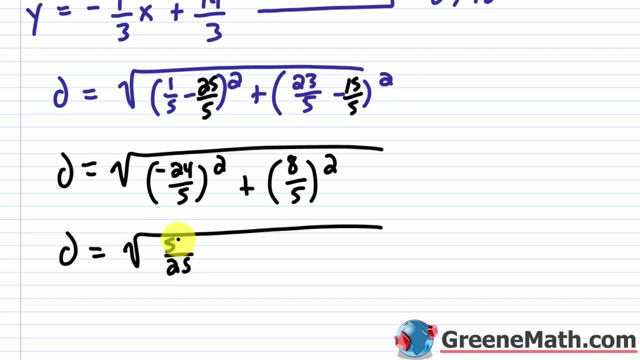 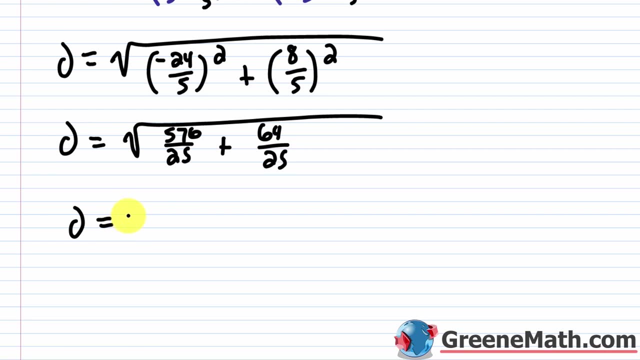 If you square negative 24, you're going to get positive 576.. So then plus this would obviously be 64 over 25.. If you want to add these two together, because you do have a common denominator, you would have 576 plus 64, which is 640.. So the distance is equal to the square root of. 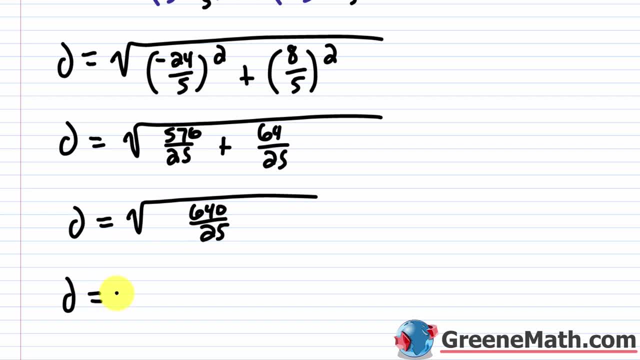 640 over 25.. So, just simplifying this, the distance is equal to the square root of 640 divided by five is 128.. And then 25 divided by five is five. Okay, So this is a little bit more manageable, something you could probably do without your calculator. So you know, 128 is. 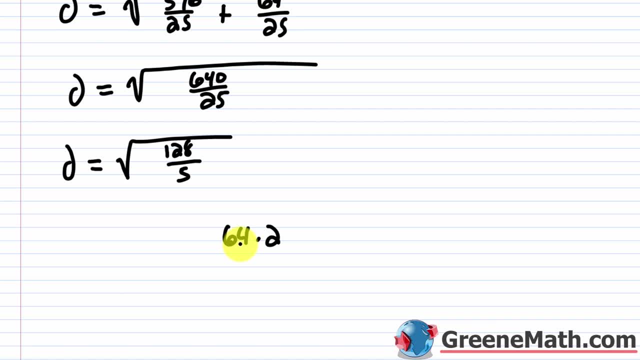 64 times two, and 64 is a perfect square right. It's eight times eight. So I could say that the distance is equal to. I'll go ahead and say: first, let me break this up and say: this is the. 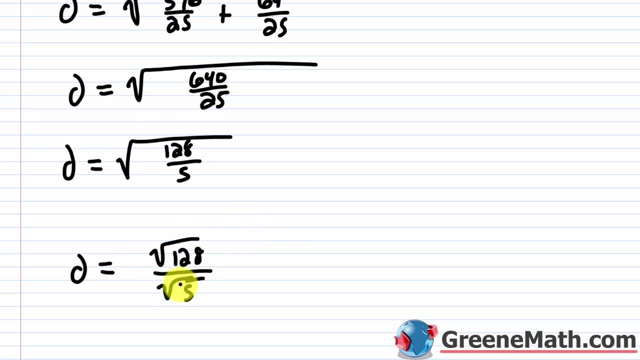 square root of 128 over the square root of five. Okay, So we have this established. Then let me write up here, Let me make a little border. I'll actually do this in a second, So I'm going to do a different color. I'll say that the distance is equal to. this is going to be eight times the. 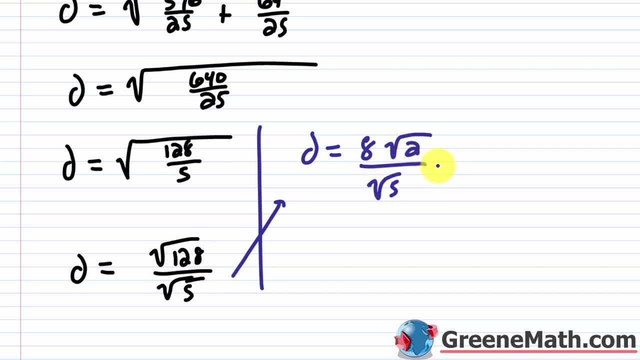 square root of two, And then over you have the square root of five, And then I'm going to rationalize the denominator, Okay, Just like we did before, And basically I'm going to end up with a distance that is eight times the square root of 10 over five. Okay, So the same answer. 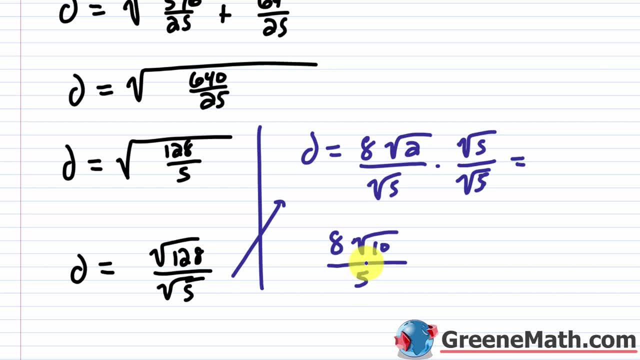 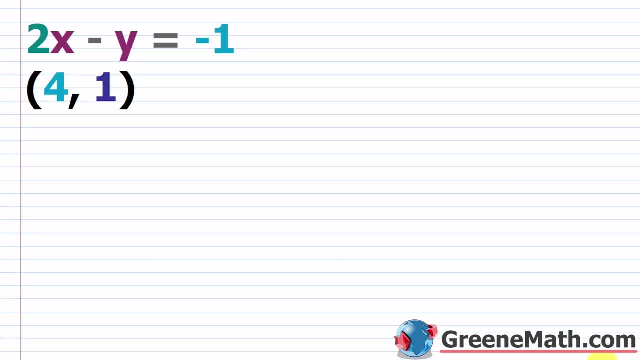 we got before. obviously it took way longer, but hopefully this gives you a little bit of insight into where that formula came from. All right, Let's just take a look at one more example. We'll do this the short way, using the formula. Obviously, you can pause the video and try this. 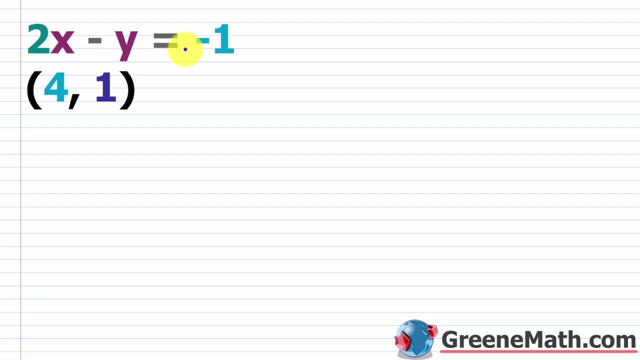 the long way. That's up to you. So we have two X minus Y equals negative one. So I want to write this as two X minus Y plus one equals zero. So very important to do this. This is your A, this is your B. It's going to be negative one again. And then this is your C: Okay, 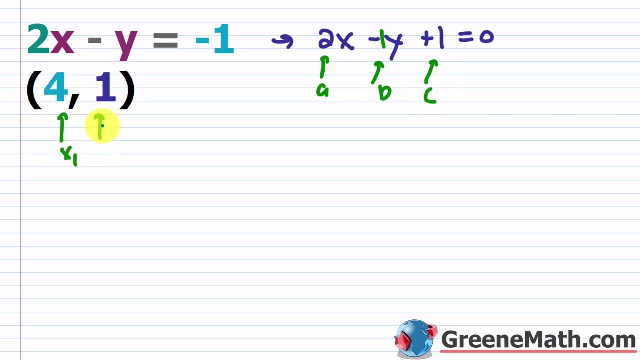 Then your point here, four, comma one: this is your X sub one. This is your Y sub one. Okay, So the distance is equal to go ahead and plug in. So you have the absolute value of A, which is two times X sub one, which is four. Then plus, you have B, which is negative one.